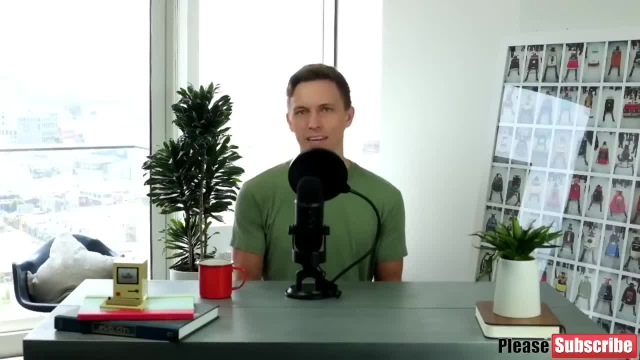 Hey everyone, welcome to the Ultimate MySQL Developer Bootcamp. I know it's a bit of a mouthful of a title. My name is Colt. I'll be your instructor for this course. So in my experience, the first couple minutes of any course- sometimes the first day of a college lecture- is all devoted to introducing the instructor, talking about the syllabus and talking about TAs and exercises and turning in assignments and you don't actually get to cover much of the content that you care about. 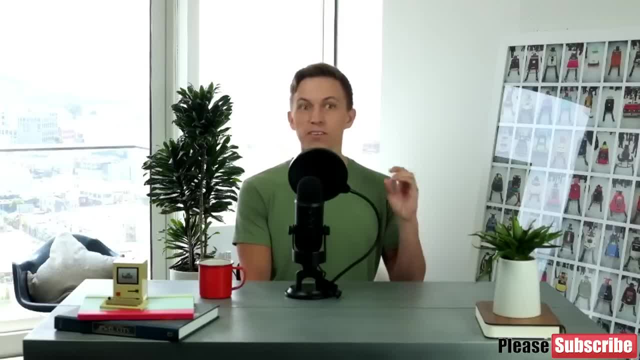 But this is a MySQL course. I want to talk about MySQL as soon as possible. So here's the promise I'm going to make you. I'm going to talk about who I am and my background, if you care about that. I'm going to talk about what the course covers, what it doesn't cover. I'll show you the projects and the assignments- all of that fun stuff, in just the next four minutes. 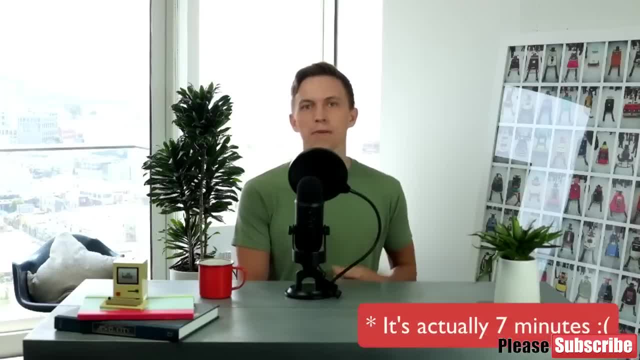 And then by the next five minutes, by the fifth minute of this course, we'll be typing SQL code. We won't have to install anything, we won't have to get set up. We have this nice workaround in the browser where you'll be able to actually run code immediately. 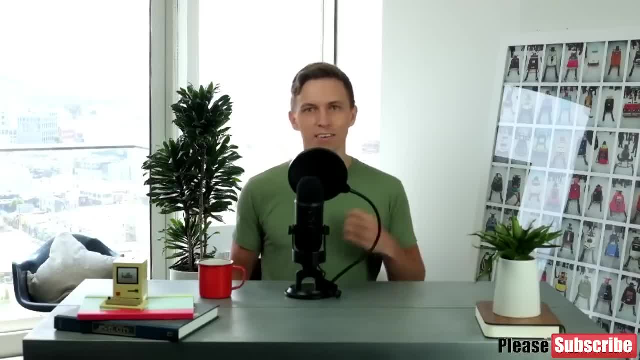 Okay, so that's my promise to you. With that said, I'll shut up. I'll start talking about myself and who I am in the next video and then we'll move on with the syllabus and so on. But remember- end of this section- we'll be typing code. Alright, let's get started. 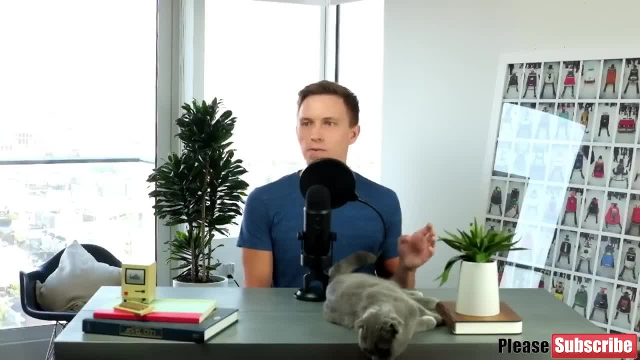 Hey there, welcome to the next video. So in this video, all I'd really like to do is spend a couple seconds introducing myself as well as introducing Blue. this is our course, TA. You'll see her pop up a couple times in the course. Hopefully you don't have a problem with cats. 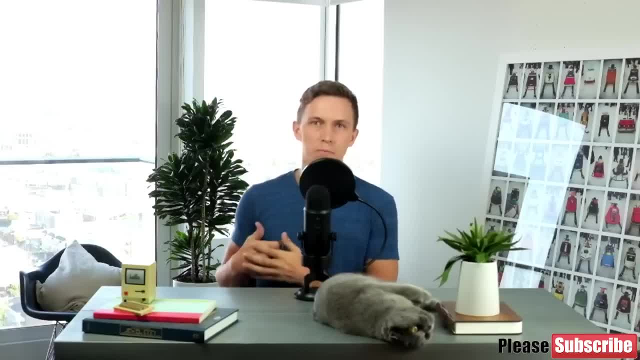 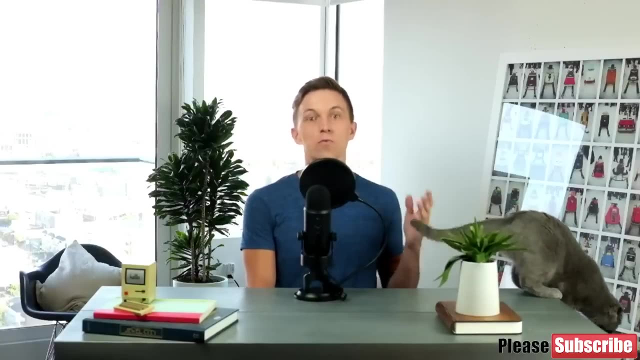 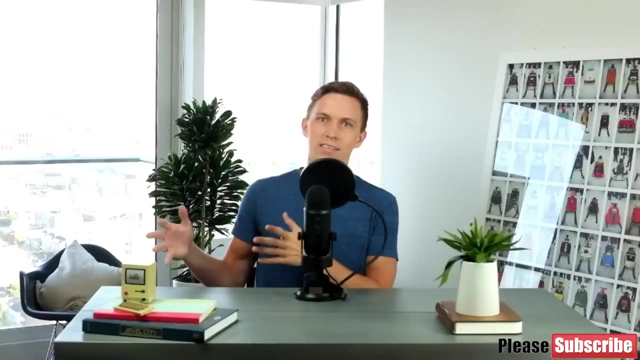 Anyways. So my background really is that I've been teaching people to program in person for the last five or so years. I've been teaching web development boot camps in the San Francisco Bay Area pretty much non-stop. So if you're not familiar with boot camps- web development camps- that is the way that they typically work- is that they're three to six month long programs where students basically commit their lives for that duration to learning to code and nothing else. 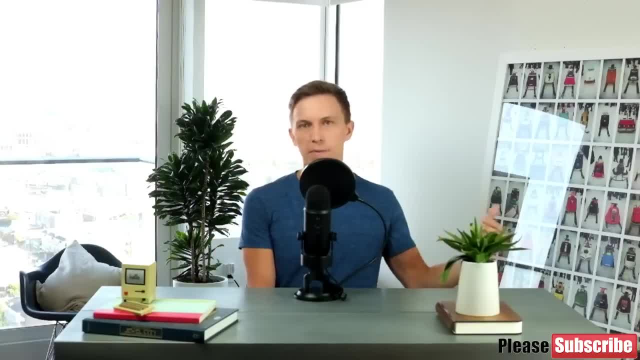 It's a very, very intense program. We take students who have zero programming experience all the way up to the point where they get it Okay, so let's get started. So this is my second course and this course, as you know, is on MySQL. It's kind of the next logical step to teach online. So I used to teach this in person as well. I'm now trying to take my curriculum and bring it to the classroom online. 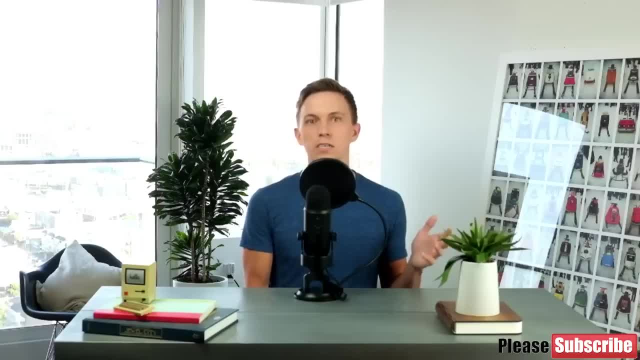 All right, so that's enough about myself. If you do have any questions, if you're curious or you're actually interested in learning more about web development, please feel free to reach out to me. If you have questions, absolutely reach out to me, Send me a message or post a question on the discussion boards. 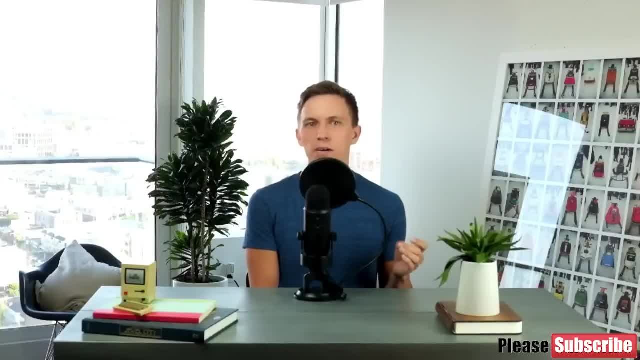 All right, see you in the next video. So what I'd like to do in this video is take a quick tour or walkthrough of the syllabus, talk about the curriculum, what the course covers and what it doesn't cover, And at the same time, it's a good place to talk about prerequisites, if there's any experience you need for this course. 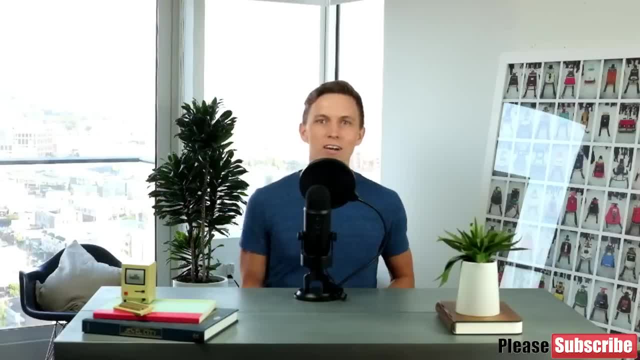 And the short answer is no, but there's a longer answer. There are a couple things that might be helpful. to do this, rather than just talking to you sitting at my desk, is to actually use the magic of editing very high tech fancy skills here and hop into the syllabus now and just go over some of the details. 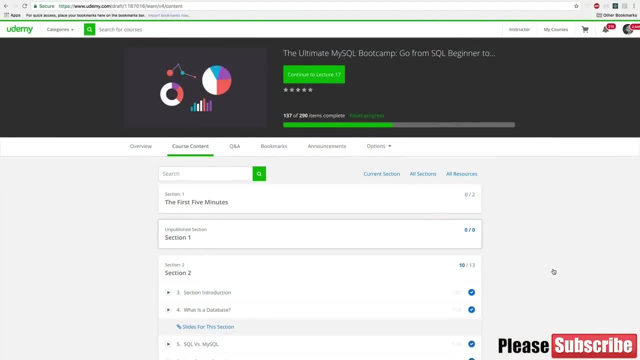 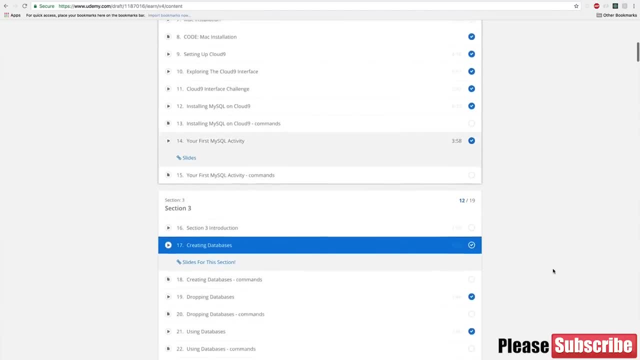 with you. all right, i'll see you there, okay, so i'm looking at the syllabus here. there's currently 300 or so different lectures across 17 different sections and i won't waste your time going over every single section. i just want to point out some of the big trends and kind of where we're going. 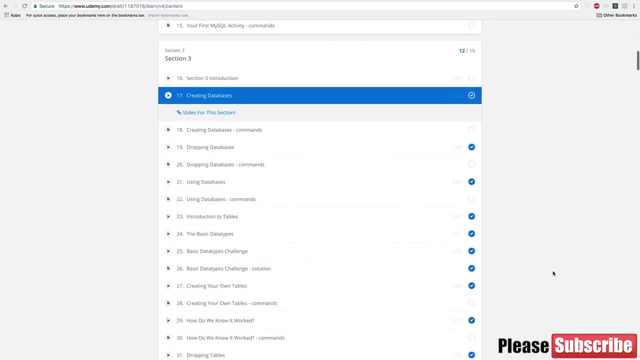 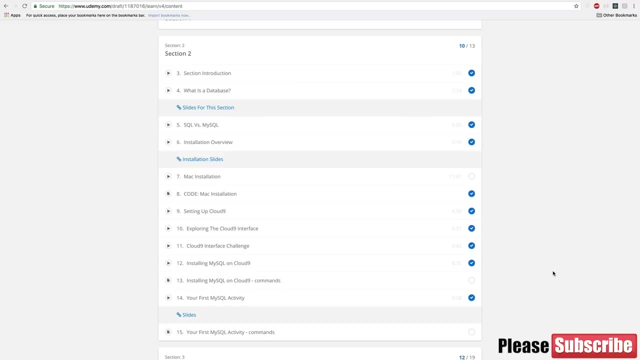 based off of where we are right now. so the next section is really focused on setting the stage for what mysql is, how it compares to other databases, what makes something a database, what sql compared to mysql, and then we shift focus to installing. so by the end of that section you'll 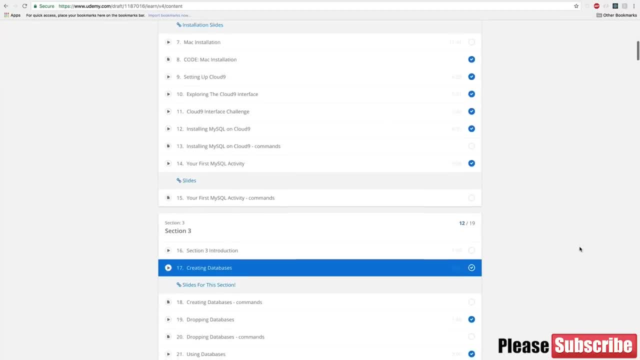 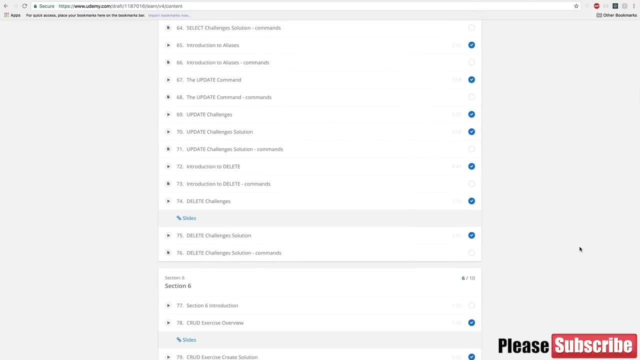 have your own copy installed and then from there we really dive into code. we see how to create databases, how to put data in there, and then we focus a lot of time on how to get data out. how do we write complex queries? and, along the way, we focus a lot of time on how to get data out, how do we write complex queries, and along the 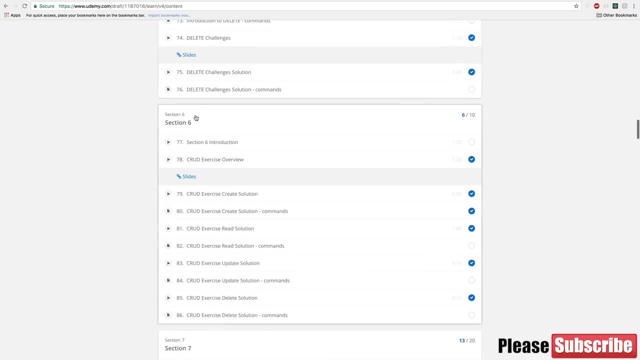 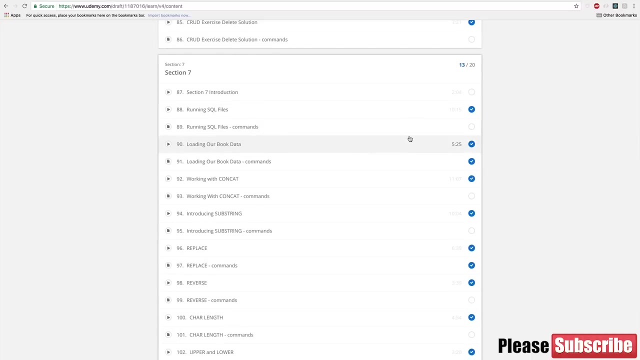 way. there are dozens and dozens of exercises, including section 6, which consists entirely of challenges. it's the crud exercise challenge, where we spend a lot of time working with one data set in detail. then we keep moving on, basically working our way up towards more complex queries, asking more complex questions of our data. so all of this, 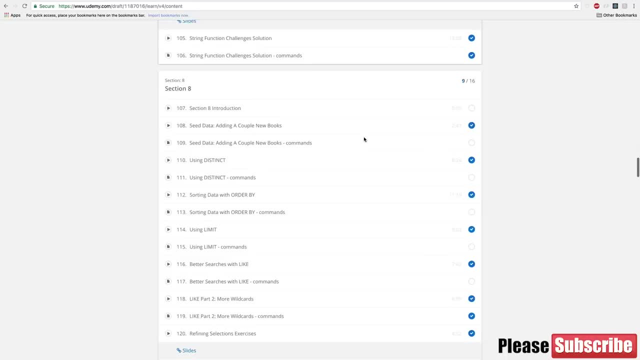 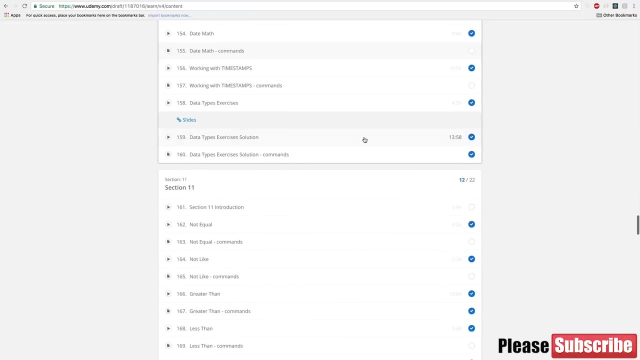 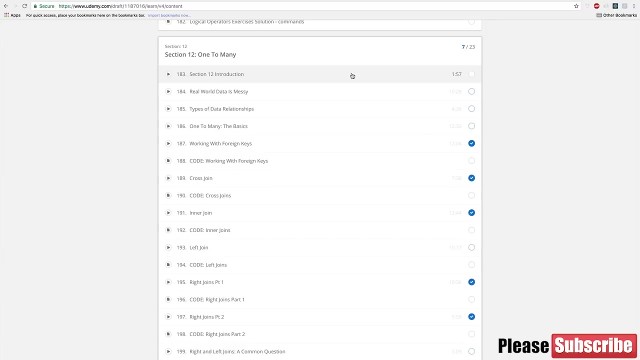 contains things like aggregate functions, learning about string functions, learning how to work with dates and date times, how to sort our results, and then also working with logical operators. and if none of that means anything to you, don't worry, but if it does, you're looking for it, you'll find it in this syllabus, and then we move on to our next chunk. 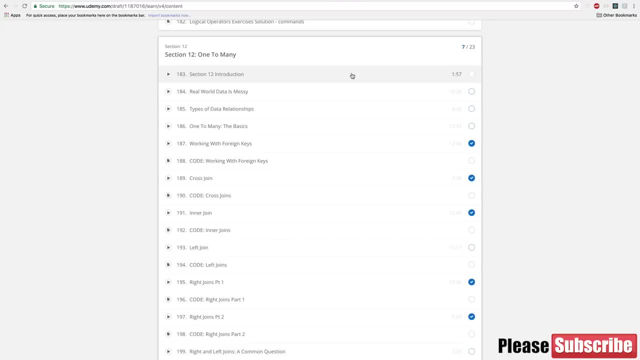 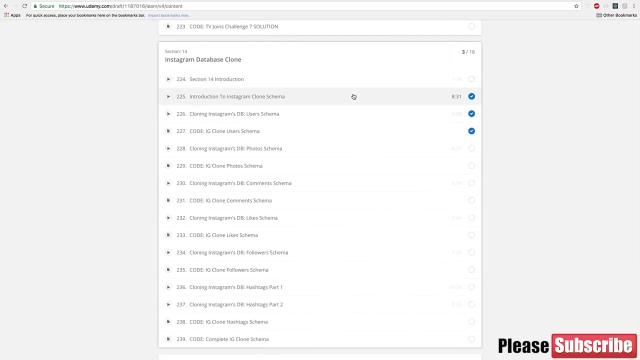 of content which has to do with interrelated data, with more complex data structures. how do we represent them? with mysql or with sql? so we start talking about joins. if you've heard of joins before, sections 12 and 13 focus on joins, and then, in section 14, we start working with our instagram. 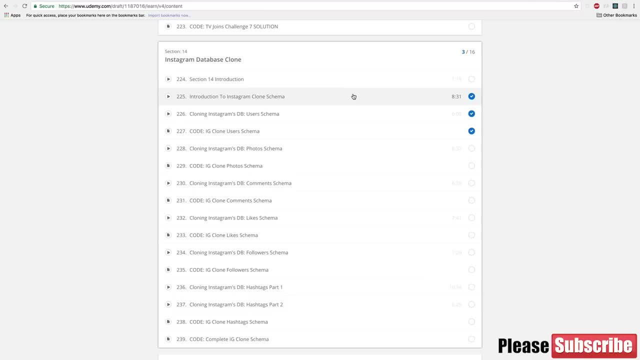 database clone. so what we'll do here is add a database clone and then we'll start working with our database clone. so we start working with our database clone and then we'll start working with actually set out to come up with a clone of an instagram like database. obviously it won't be. 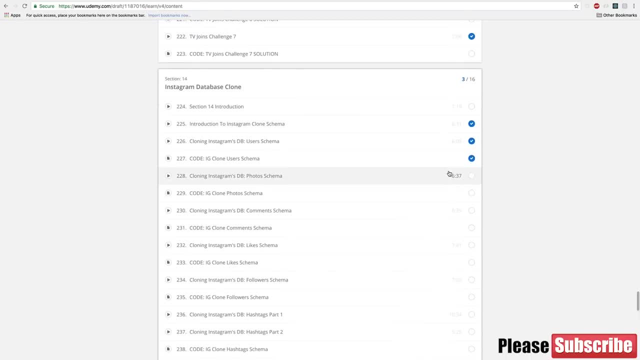 as complex as instagram, but we work with things like photos and users and comments and likes and hashtags and followers and friends, all that fun stuff. so we'll set up our database here, we'll design it and then section 15 is all challenges using that instagram data. so it sort of serves. 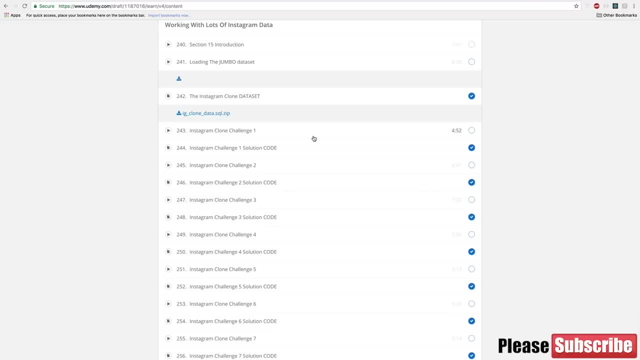 as a final exam to the course, although not a test- there's solutions immediately after- but it sums up what we've done until this point. you'll have a bunch of data, thousands and thousands of rows of data- that i'm going to provide you. you'll put it in your database and then you'll write code. 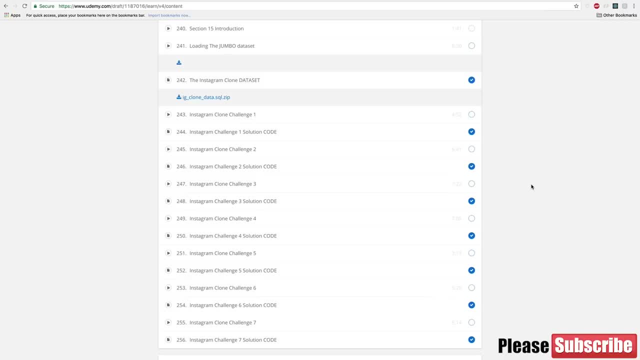 to answer a bunch of real world questions that someone or some company might have about the data. but that's not the end of the course. we move on at the end into kind of a broader section where we start talking about mysql plus other languages, so we see how to interact with node. 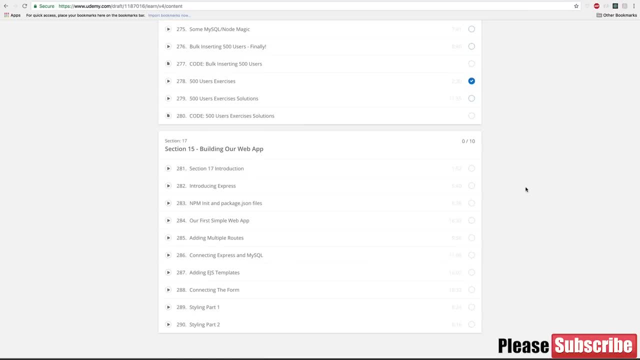 in mysql and then finally, the course ends when we build a simple web application using mysql and nodejs together. so that's a rough overview of all that we cover. one thing you might be wondering about are the prerequisites, and i did say earlier that there are no prerequisites. you 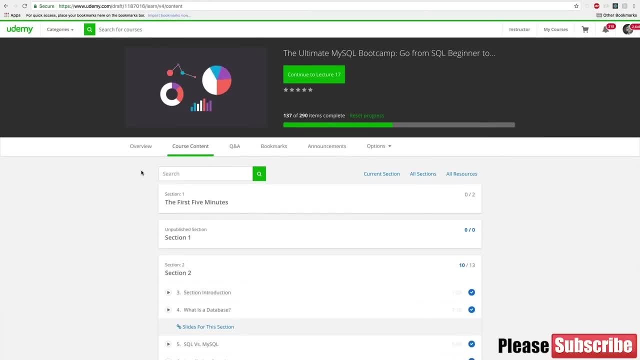 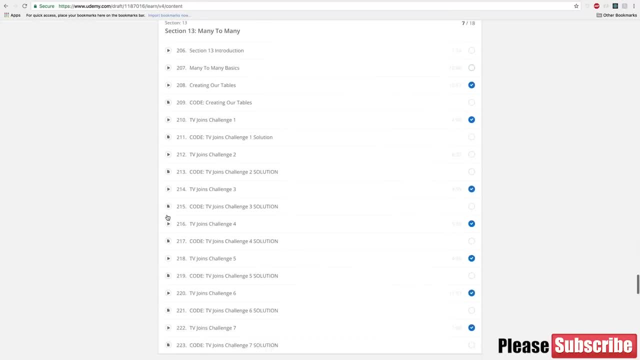 don't have to have any experience aside from being able to work with a computer, being able to work the internet, download things. but i should note that towards the end, well, at the very end, when we start talking about nodejs and building a web app, it definitely will help. if you're. 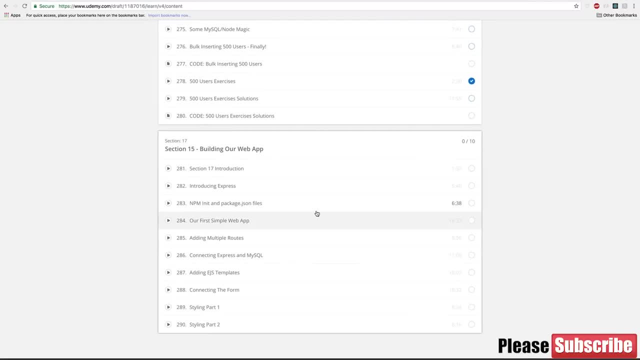 familiar with things like javascript, html and css. this isn't a course on those topics, so i'm not. i don't spend, you know, hours and hours going over them like i could. however, i do spend a little bit of time introducing them. you know, in a couple minutes doing a crash course, but that's not. 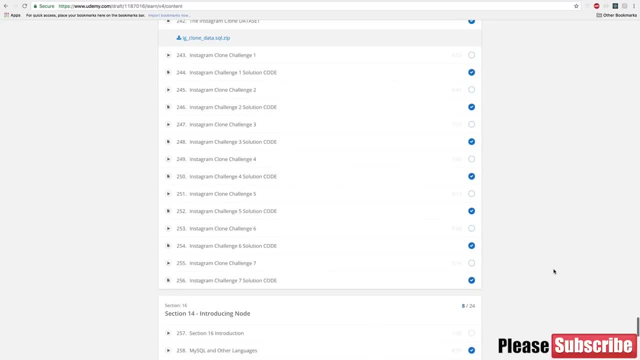 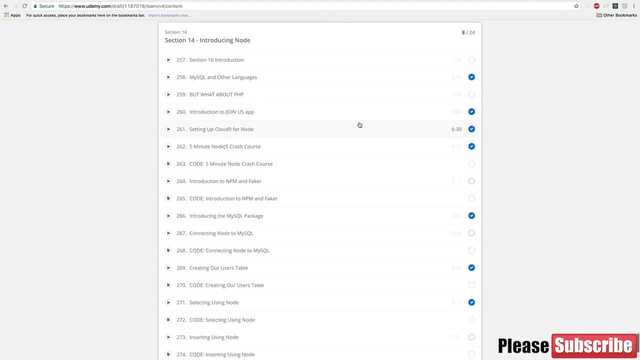 the focus of this course. so that's the only note i would add. if you're here just for mysql, and that's what you're concerned about, there are no prerequisites. but if you really want to be able to understand nodejs at the end and the web app that we build, it will help if you have. 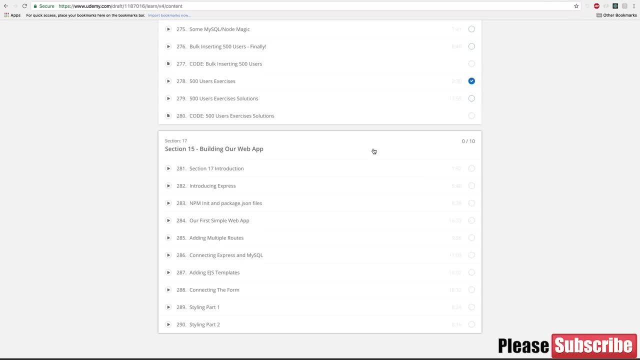 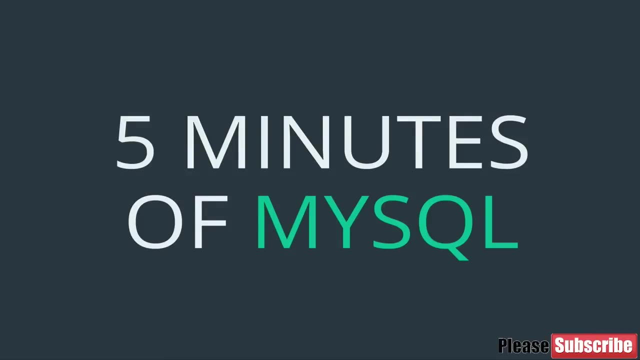 a little bit of experience with html and css and javascript. other than that, though, no prerequisites i mentioned- i wanted to get us writing some code as soon as possible, so that's what we're going to do in this video. obviously, it's super early on in the course, so don't get your hopes up for doing. 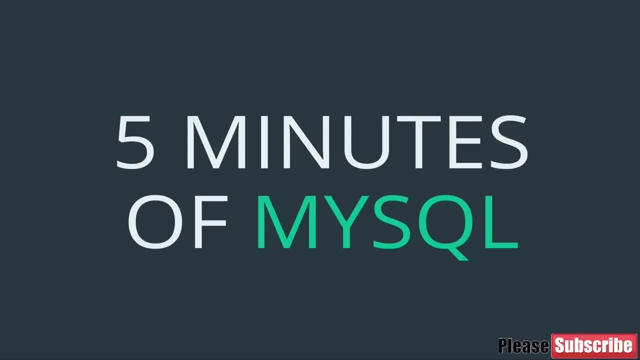 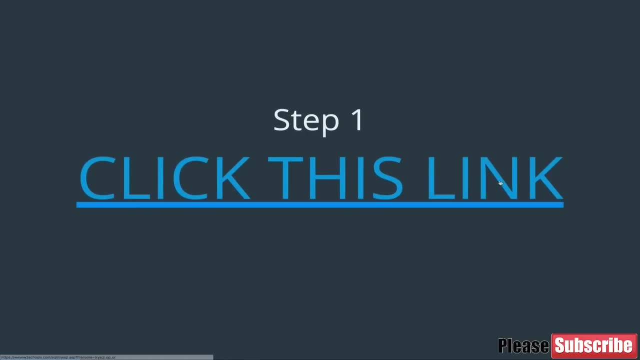 anything crazy impressive. it's going to be pretty basic, but the idea is that i just want to introduce you to writing some sql, show you what it's like. so the first thing you'll need to do is click on this link if you want to open the slides. i've included them with this lecture, or i've included 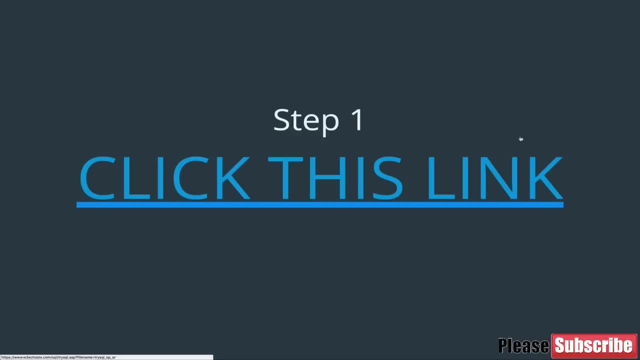 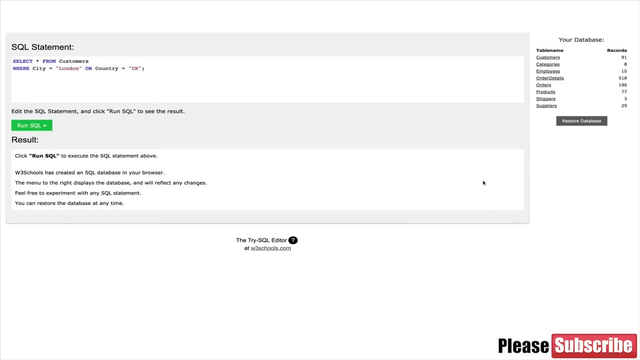 the link itself as a resource with this lecture. so, however you would like to get there, go to this link, which takes us to this page right here. this is the try sql editor, and i'm going to make my screen a little bit bigger just so that you can see it. here we go, and i'll start by just deleting. 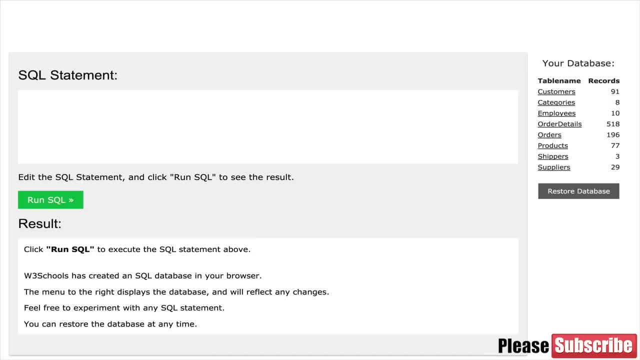 what's already in there. so you might be wondering: what is this place? that's a good question. it's an interactive browser-based sql environment, and what that really means is that think of it as your own personal sql sandbox in the browser where you can go try some things out and play around. 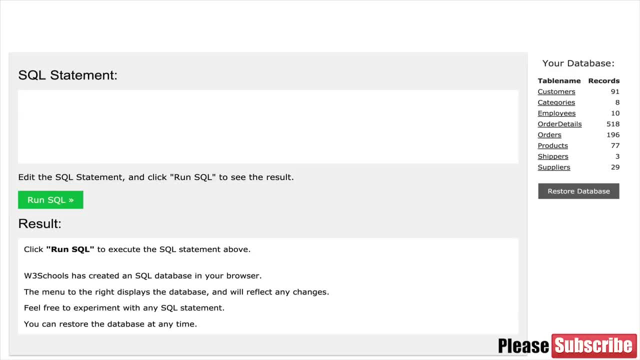 it's purely for educational purposes. so this is not what you would be doing if you were actually working with a real production database. But what it lets you do is type some SQL queries and run them by clicking this run SQL button and you'll get a result, And that's fundamentally the. 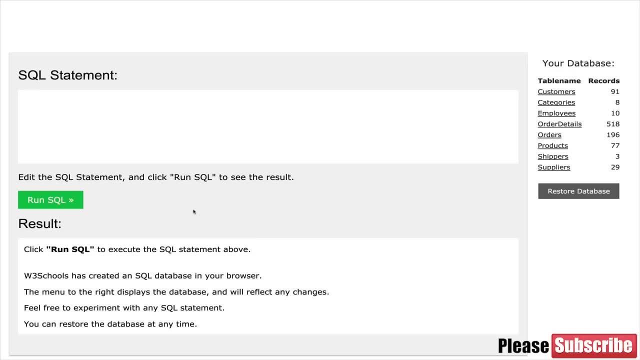 process of working with SQL. You type something and then you run it and then you get something back. Oh, and before we go any further, I should point out that we're talking about SQL here, not MySQL yet, And if you're confused about that distinction, totally normal question to have. 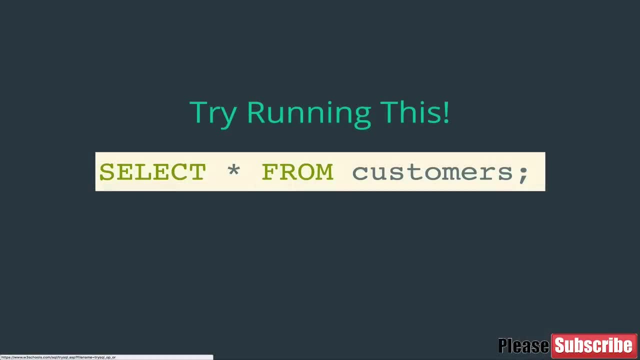 wait until the next section when I go into detail about the differences, But for now I'd like you to try running some code. So here's the first line of SQL that we can try running: Select star from customers. So you can either type this or copy it from the slides or from: 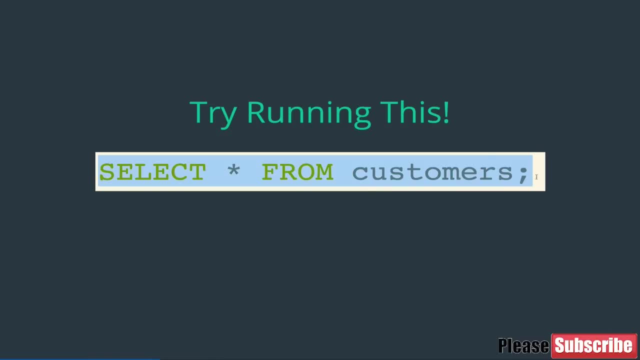 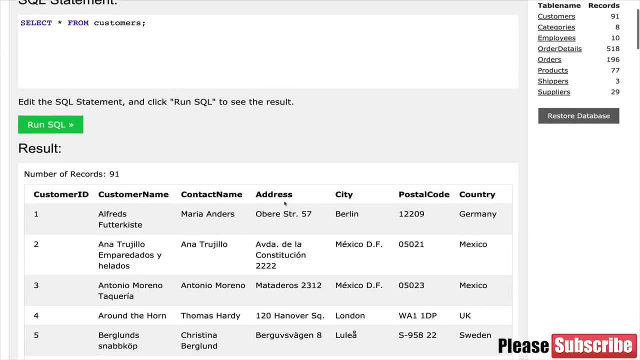 the included code file after this lecture. So I'll just copy it from the slides here And then back in the editor. I'll paste it in and click run. So the first thing you'll notice is that we get a bunch of data back. So I'm not going to go into the details of the syntax and what all. 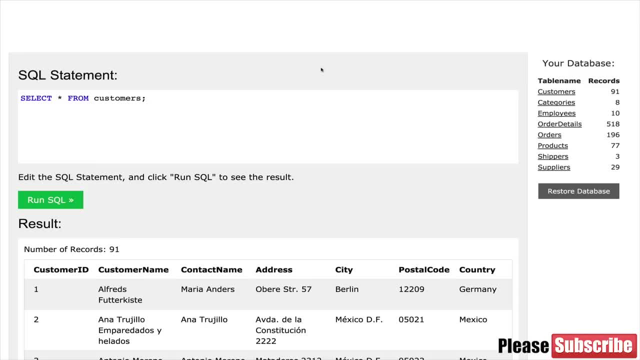 this means for every command we run. It's really more about just giving you an experience of running a SQL, So I'm going to go into the details of the syntax and what all of this means running commands. The rest of the course talks about the details in the syntax, But what this? 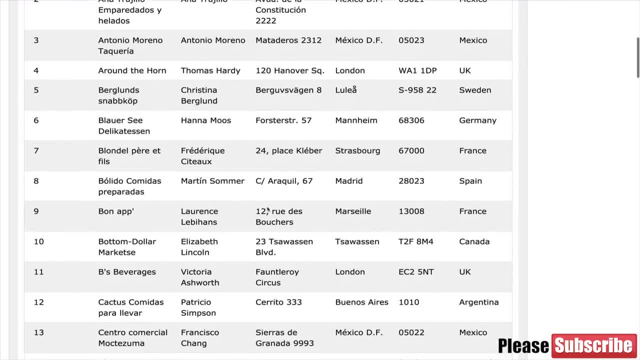 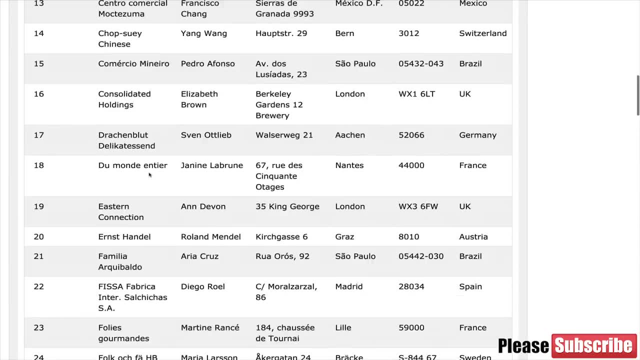 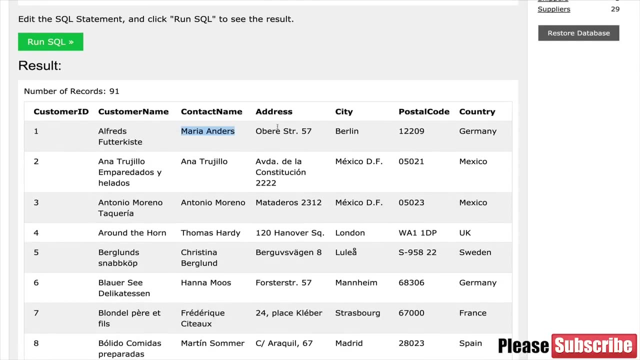 does is it gives us all of the data about customers in this database. So you can see we've got 91 customers and every customer here has a name. So these are stores or restaurants. There's the contact at the restaurant or at the business, the address, the city, the postal code and the 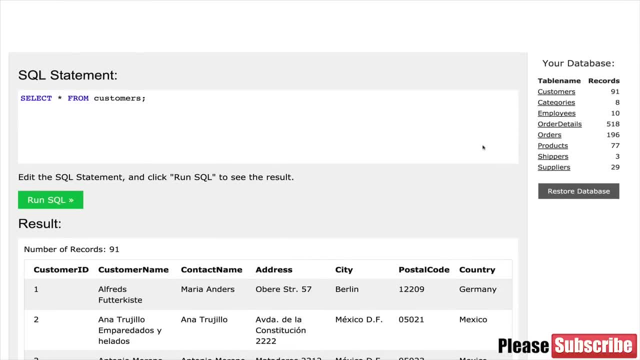 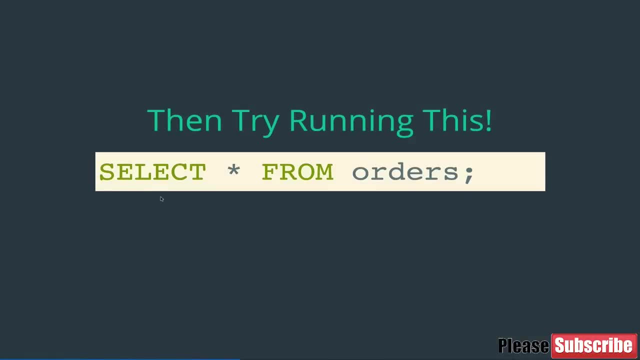 country. Okay, so that's all I'll say about that. Select star from customers. That gives us all of our customers' data that are in the database right now. So here's another thing we could try. It's very similar Select star from orders. So we'll just copy that And back here in the editor. 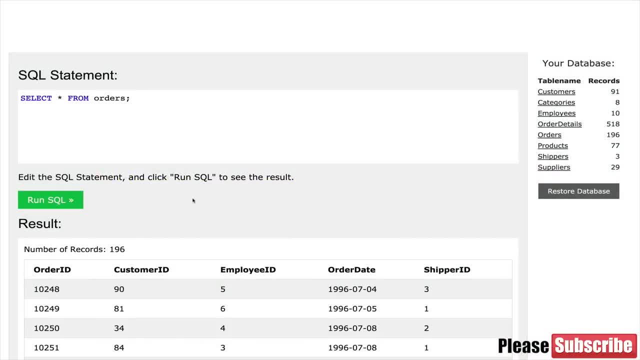 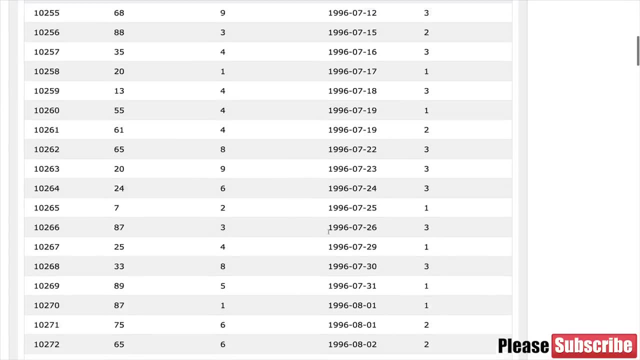 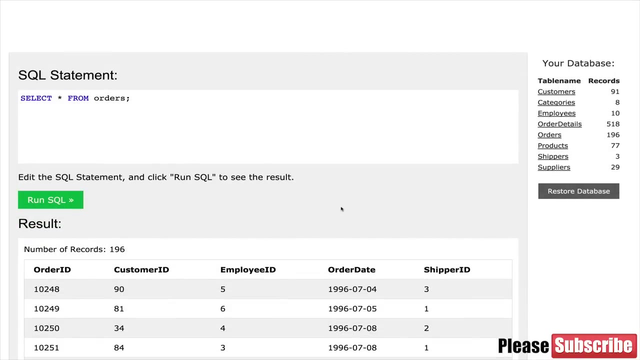 I'll paste it in and click run SQL. run SQL. Same thing happens, but this time we get all of our data printed out for our orders, So you might be wondering where is this data coming from in the first place? Very good question. It's pre-programmed in here, So every time you open this in your 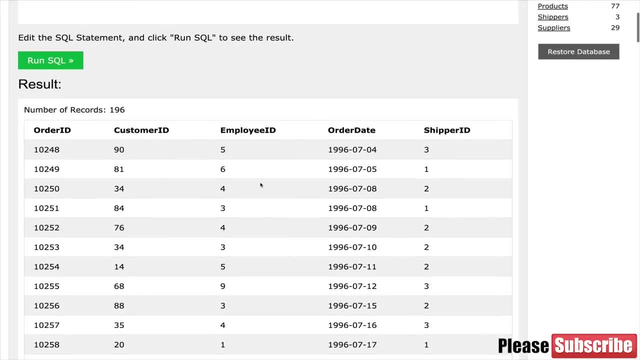 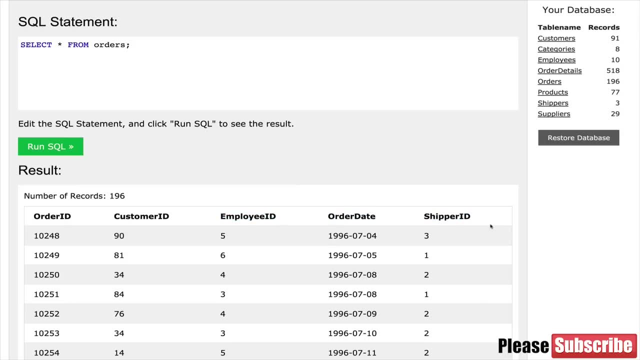 set that you can work with And just by taking a quick look at our order data, you can see we have things like an order ID, a customer ID, an employee ID, an order date and a shipper ID, But there's. 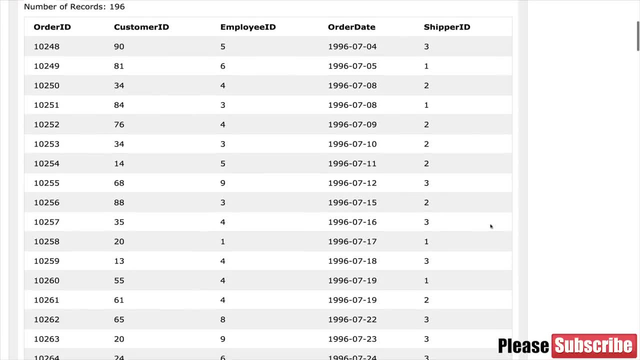 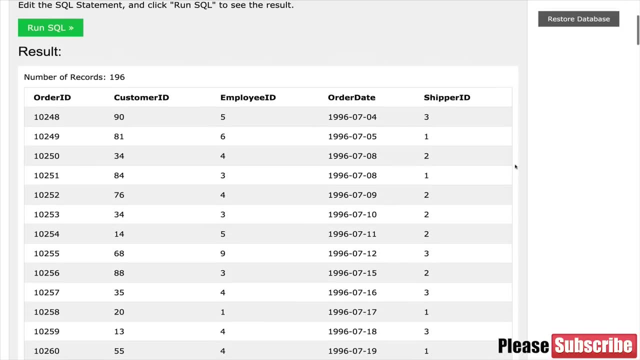 really not much descriptive information here, And that's actually why I chose this table. I wanted to make the point that a lot of the data you'll be working with on its own or like a snapshot like this, isn't very meaningful. What we actually want to do is start combining it with other tables. 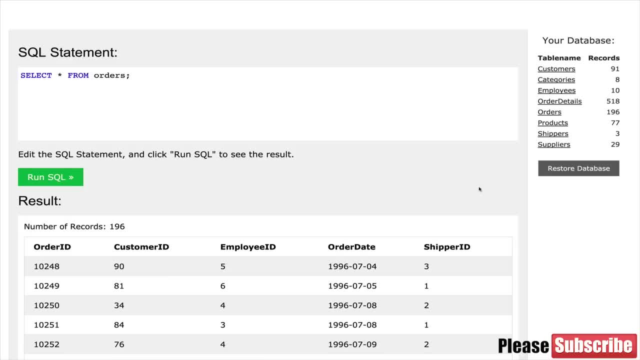 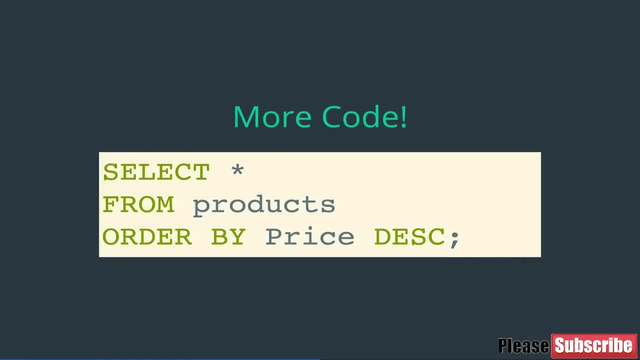 So we're not going to do that now, but that's what we're building up towards the end of the course is to combine customers with orders and products and shippers to get some meaningful answers out of my data. So here's another thing we can do, very similar to what we've done already, but there's a. 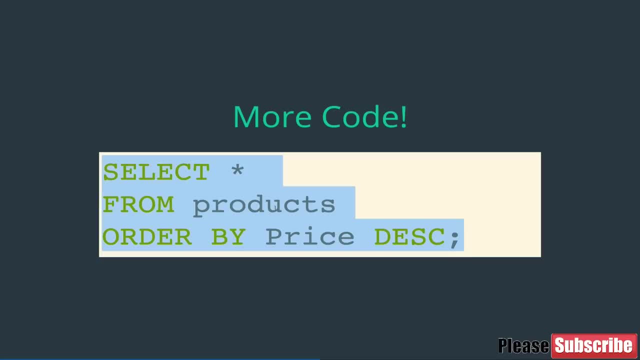 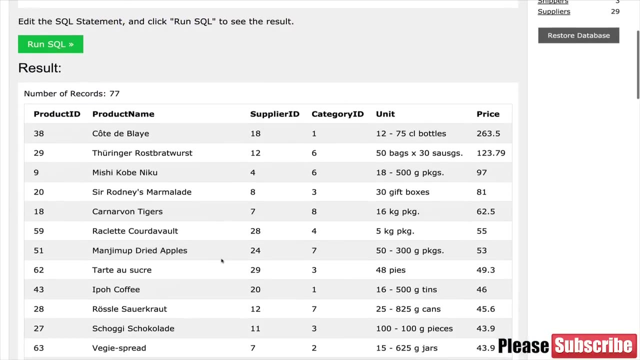 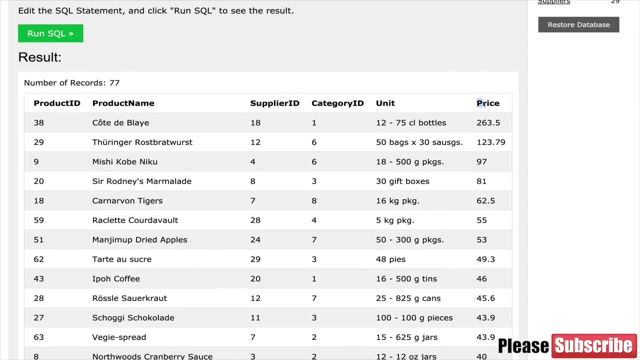 little bit extra. So select star from products order by price descending D-E-S-C. And if I paste that in here and click run, what I get now are all of the products in my database. So they have a product ID, a name, a supplier ID, category ID, a unit and then a price, And they're currently 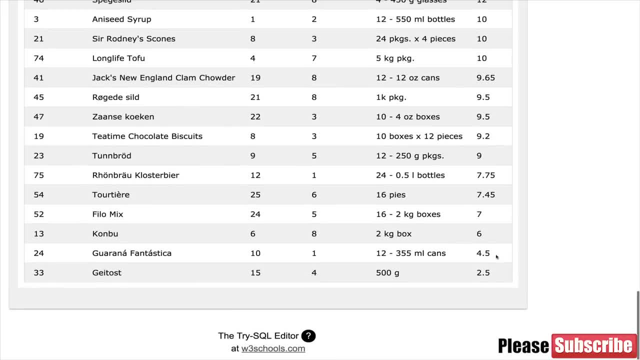 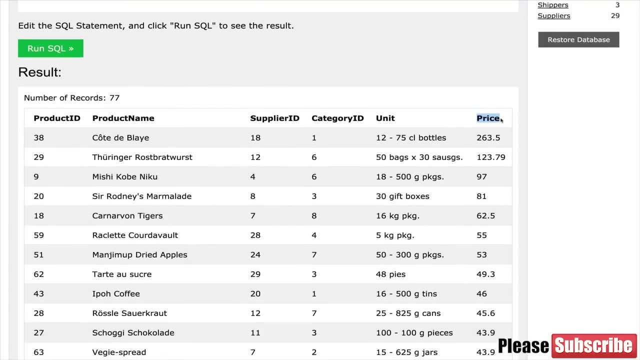 sorted by most expensive down to the cheapest, all the way at the end. So I won't force you to listen to me trying to pronounce some of these, but these are our products and they're currently sorted by price. So just a simple modification to the query yields radically different results. And if we just 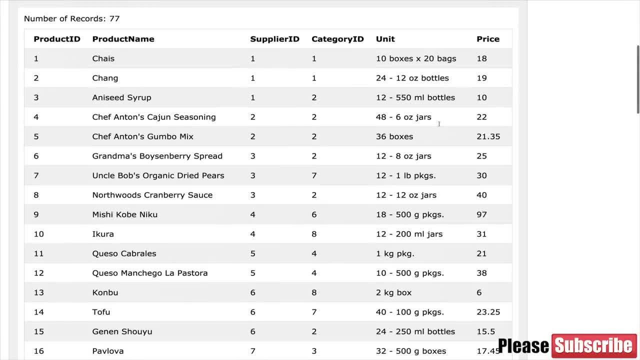 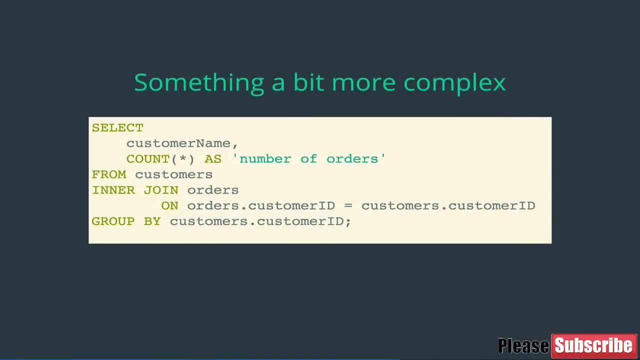 get rid of that order by price. we get the same data back, but now it's ordered by product ID rather than the price. Okay, And stepping up in complexity a little bit here, here's another query, this one significantly longer, And this one actually involves: 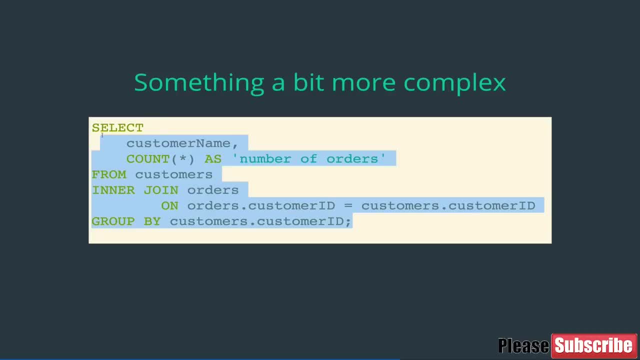 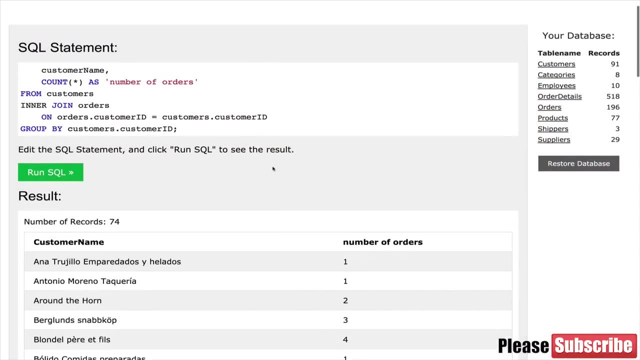 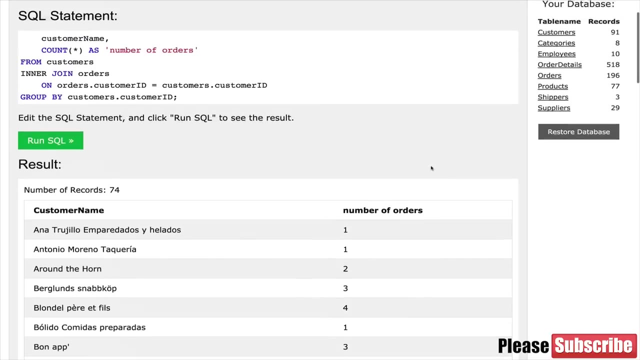 two different entities. So we saw customers, we saw orders separately. If you try copying this and pasting it in and you click run, what we actually get here is a list of records for a customer And then the number of orders a given customer has placed. So remember, this data is. 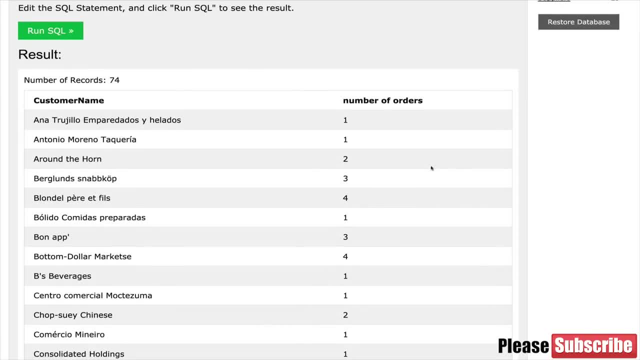 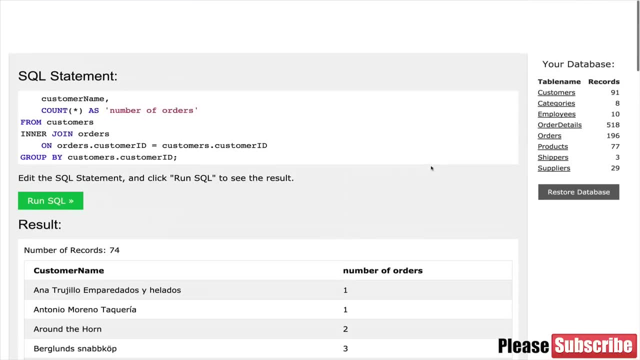 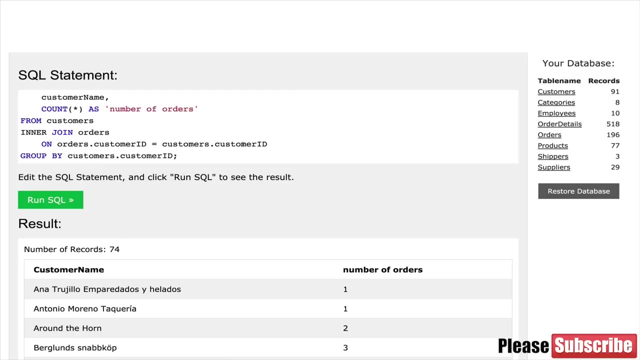 stored in two separate places. We had the customer's data that had nothing to do with orders, And then we had the order's data and all that it contained was customer ID, And then we've combined them with this query. So do not focus on the syntax, Don't panic about that. Of course we'll get there. We'll talk a lot more about how to. 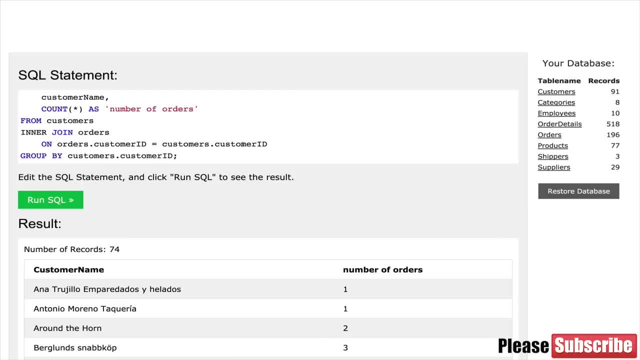 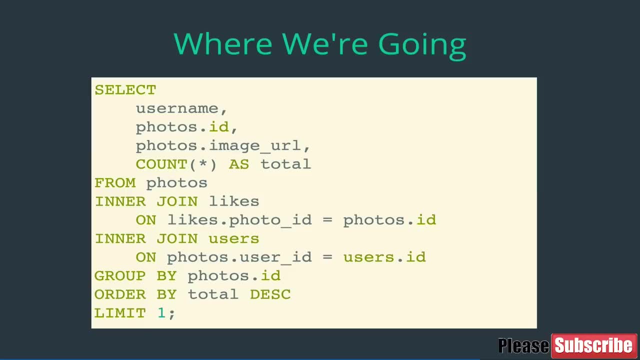 structure queries. I mean, most of this course is about structuring complex queries. In fact, here's a quick preview of some of the things we'll be doing. So here's an example of a slightly more complicated query. This time we're working with photos and images. We're working with users and likes and putting them all together to get. 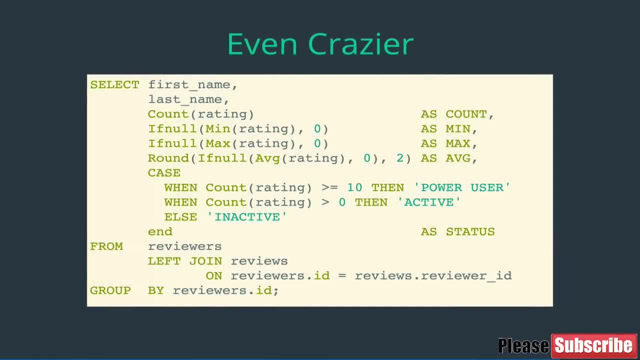 some information out, And here's another one, a little bit crazier, where we're working with ratings or reviews and TV shows and reviewers. So think of it's like a Netflix or iTunes, where you could rent or watch a TV show and then rate it. 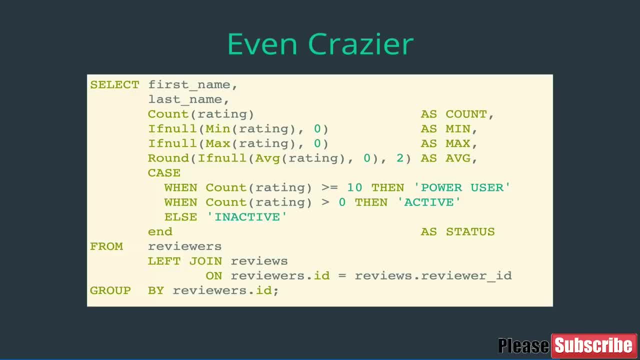 from 1 to 10 or 0 to 5, for whatever the rating scale is. Here. we're working with that data to figure out who our power users are, who are the most active users, who are reviewing the most things. So we'll be building up to these sort of queries and by the end of 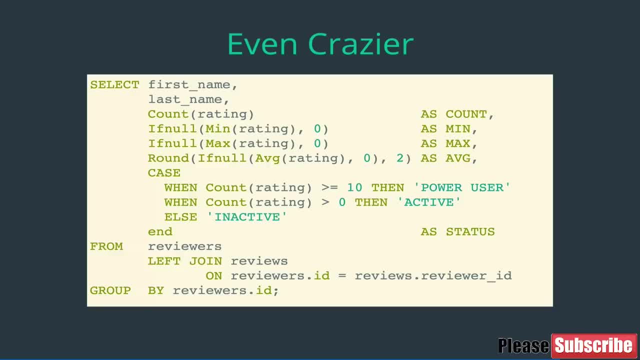 the course. you should be able to make sense of this and do a lot more, by the way. Okay, So that was a taste of SQL. Hopefully it didn't taste too bad. So in the next section we'll dive into the nitty-gritty of what SQL is and how it compares to MySQL. 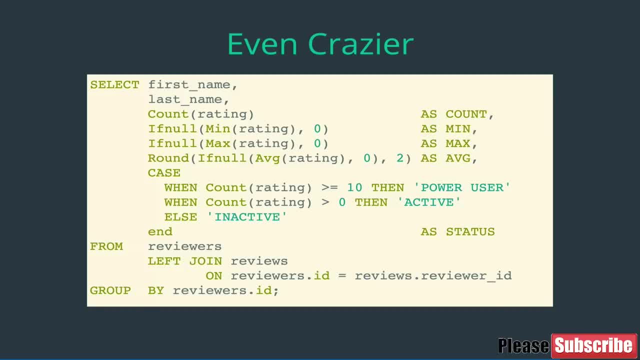 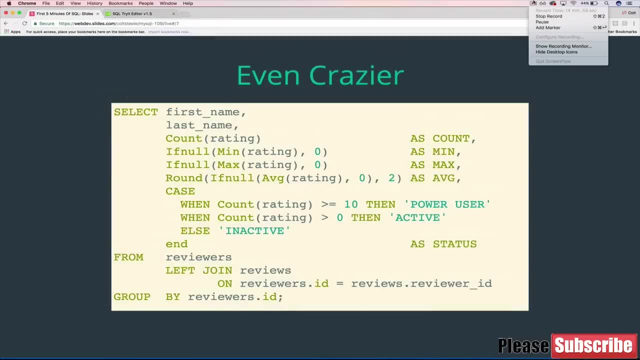 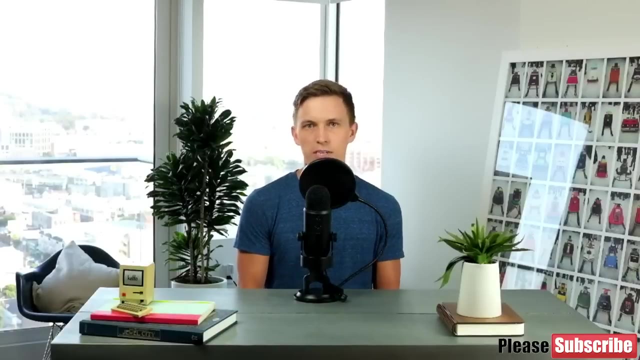 we'll get everything installed and then, finally, we'll have our first set of exercises. All right, so I have some good news, which is that in the next video, we're going to start typing code, We're going to start with SQL. The bad news is that we still have to make it through. 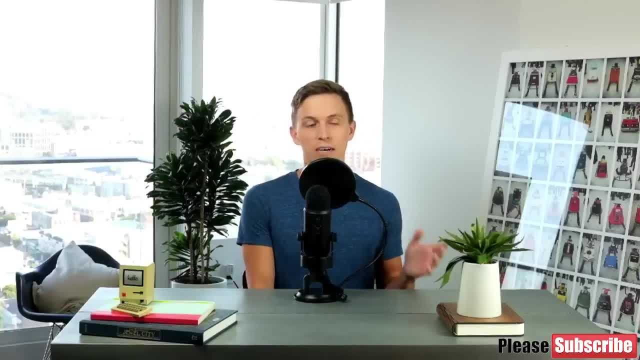 this video. Hopefully it's not too painful. Essentially, what I want to talk about is different types of content in the course and how the course really works. It might be a little different than other courses you've taken online, depending on how they were structured Basically. 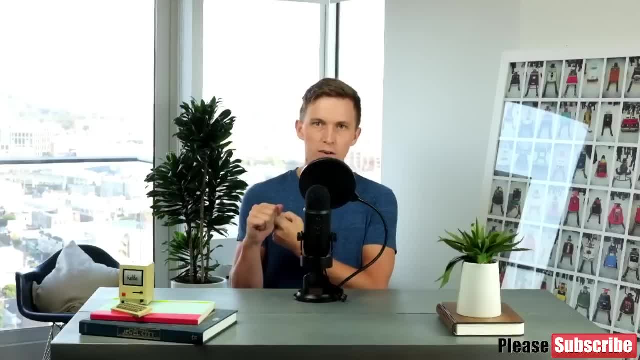 I break the content into a couple different categories. The first are things like this video, where it's a video of me talking, usually with Blue and you know what. you don't have to watch them. They kind of just serve to introduce content. It's a way for me to kind of interact. 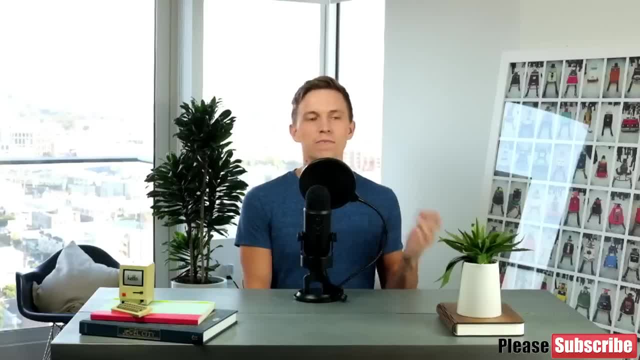 with you to say hello and to set the stage for what comes next. And if you're someone who has no patience for that sort of thing, you can do that by clicking on the link in the description: Absolutely skip it. So then, after that, we've got the actual content of the course. 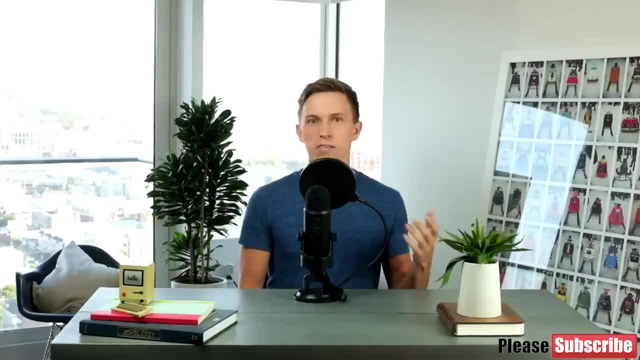 the lectures. So there are a ton of videos where it's mostly screencast and I'm explaining concepts. I usually make a bunch of diagrams, slides. I try and make things somewhat visually interesting. I'm not a great graphic designer, but I try and keep things interesting to look at. 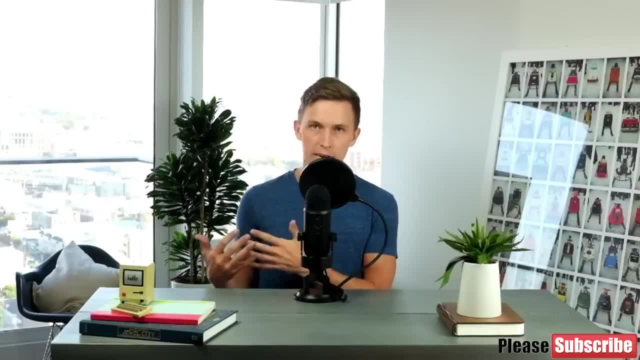 And then I also you know type code And there's a lot to watch there. ideally So, it's a combination of slides, with me talking over it, as well as diagrams and animations, and then most of the time, typing code in our text editors and running SQL code. So those are the lecture. 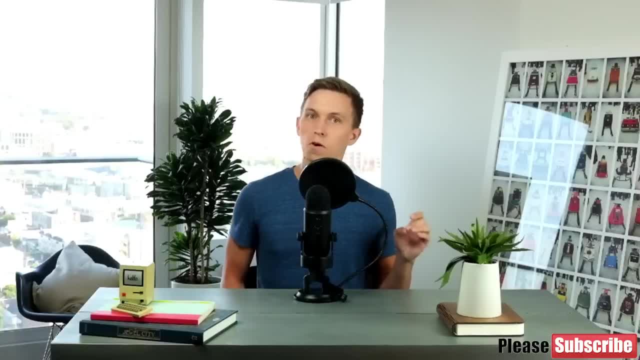 videos. But then we've also got- and this is probably the most important part, more so even than the lectures- which are the exercises. So one of the things that I think makes my courses stand out a bit- some of the feedback I've gotten has to do with exercises and activities. 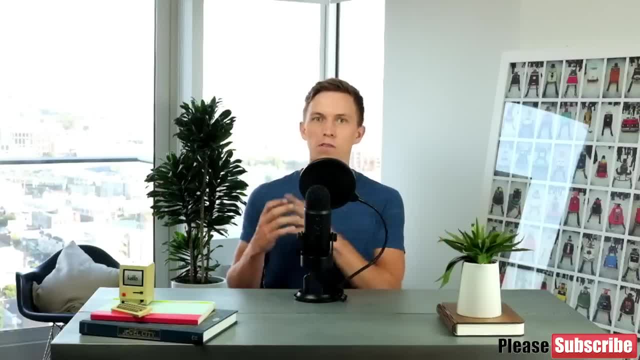 And I think they're really, really central to making a good course. So I kind of throw them everywhere in the course And then, within those exercises, we've got a couple different categories of challenges. The first are what I'd call rapid fire. basically, pause the video. I'll ask you a. 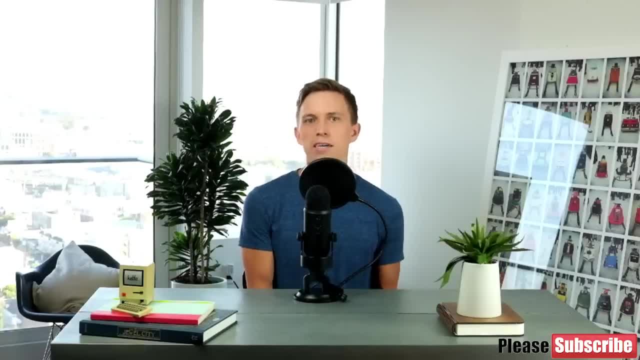 question, very short quiz type questions. And then there are the second type of exercises, which usually come at the end of a section, the last video typically, and it's an entire video dedicated to exercises. Usually there's like five to ten challenges in that video And then following that, 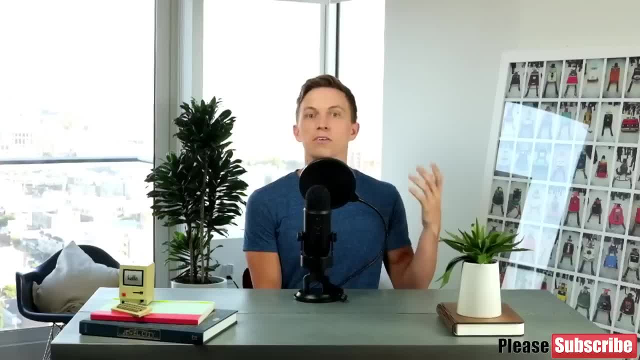 there's always a solution video where I go over the solutions, I tell you the answer and then also show you myself coding them And, as always, I'll see you in the next video. As always, the solution code is available if you don't care to see me explain it, If you just want. 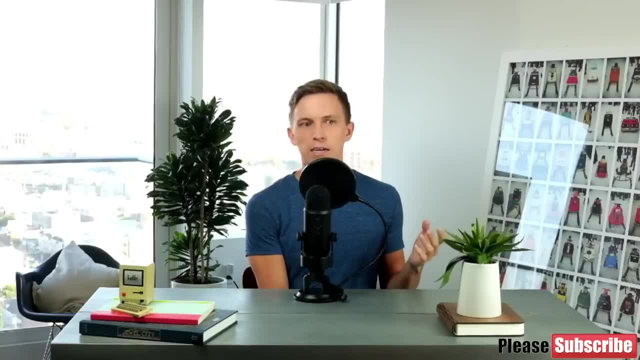 the code. you can get that at any time, And the final type of challenge is more comprehensive. So essentially, there are a couple of sections that are entirely devoted to exercises, So they might have seven or ten different videos, but they're all about one set of problems. So there's. 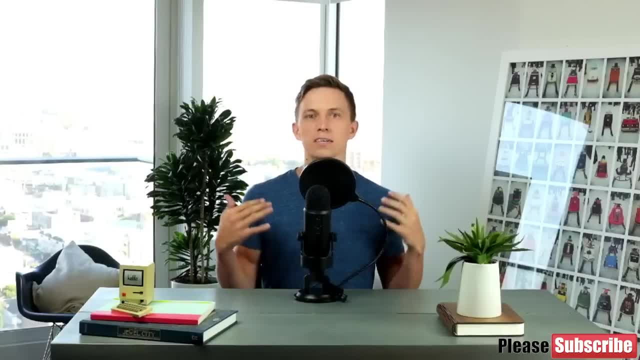 not many of these in the course. they take a while, but there are a couple of these challenge sections. So, just to reiterate, we've got quick rapid fire questions, we've got more general kind of summations, and then we've got a couple of questions that are entirely devoted to exercises. 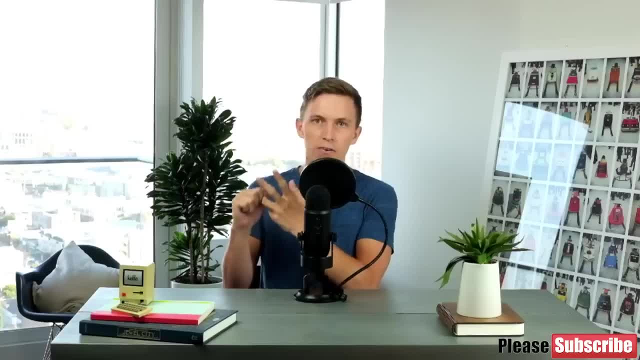 And then we've got entire challenge sections And, of course, after every lecture I include the code, all the commands that I type. they're in a file that always comes after the lecture And it always starts with the word code in all capital letters. So the last thing I'd like to add is a. 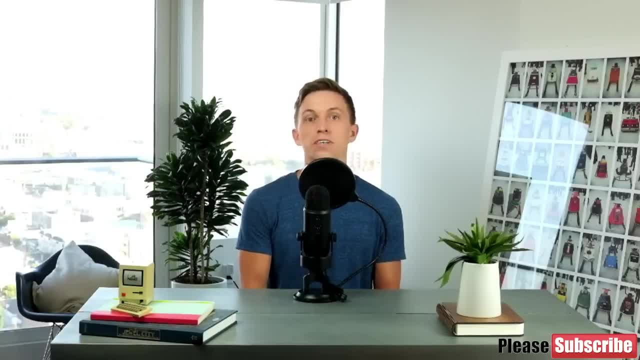 piece of advice, I guess, which is that I highly recommend you do the challenges and do these exercises. Obviously, I have no control over that. you can just skip through everything and just take the pieces of the course you need, But if you're trying to get the full experience, you can do it. 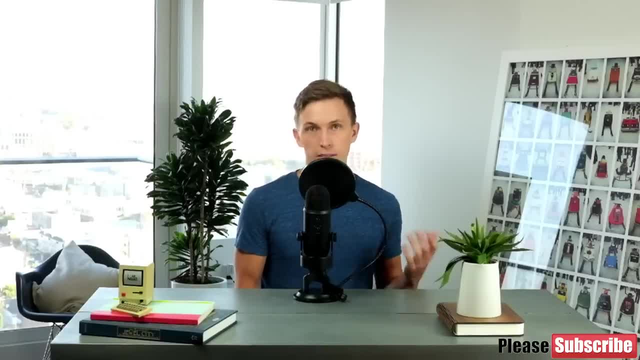 the way that I designed it. I would do all the exercises, do the challenges, even if that means you know going at a slower pace. it definitely means you'll go at a slower pace, But you'll learn much better And hopefully you'll have a better experience. And with that said, the other component. 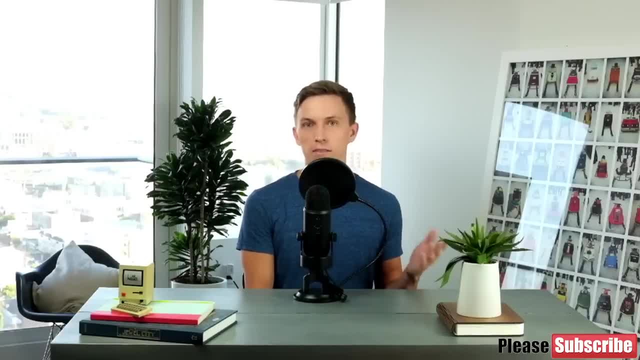 that's really important are the discussion forums. we have a full time TA in the course, as well as myself, who are here to help you at any point, So absolutely lean on that, ask any questions you can come up with. We're here to help. All right on to the course. Let's get started. All right. 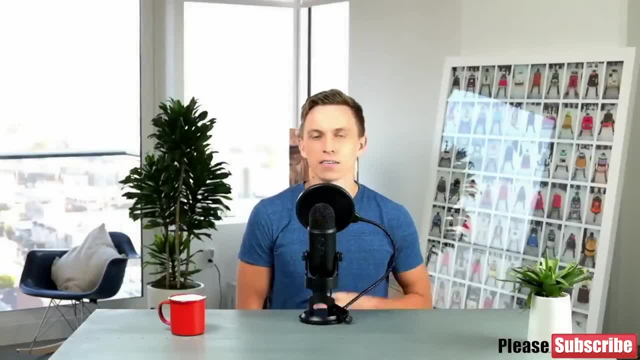 welcome to the next section. Hey there, welcome to the next section. So this section is really important. It's where we actually start talking about code, It's where we install everything And by the end, you'll be running your own SQL commands. So some big things we're doing To start. 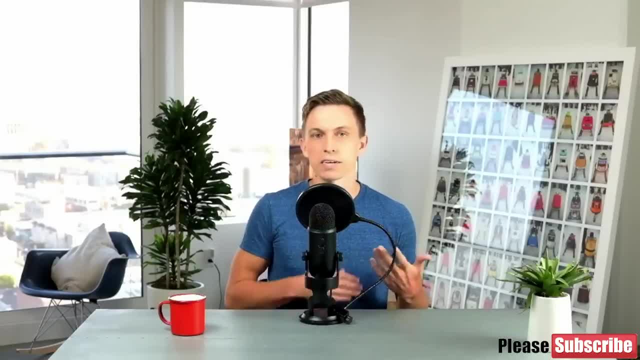 off. we're just going to talk about what makes something a database. What makes something a database compared to, I don't know, just a programming language. What's the difference? And then we talk about the difference between SQL, SQL and MySQL- a really common question. 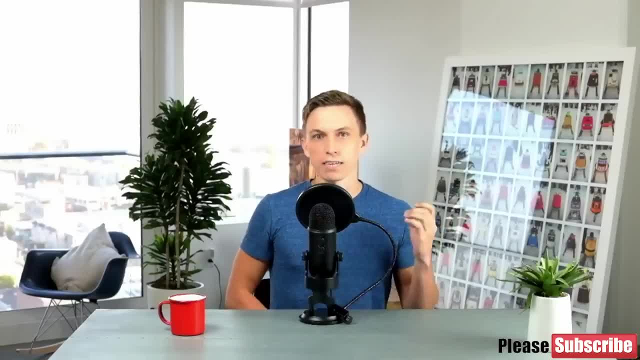 and something that's basically fundamental to all databases, or all relational databases at least, And then from there we're going to move into installing stuff. really important step for this course: you'll install MySQL, get it up and running And, by 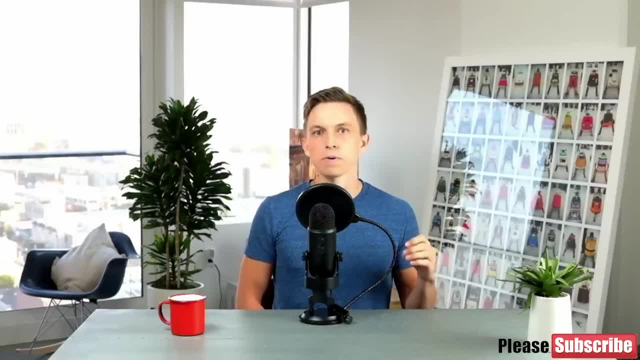 the end of the section for some of the challenges and exercises. you'll be running your first bit of MySQL code, So nothing crazy, we're not working with any. you know complex data yet we will be, but not yet. We're starting off nice and easy, just some simple commands. 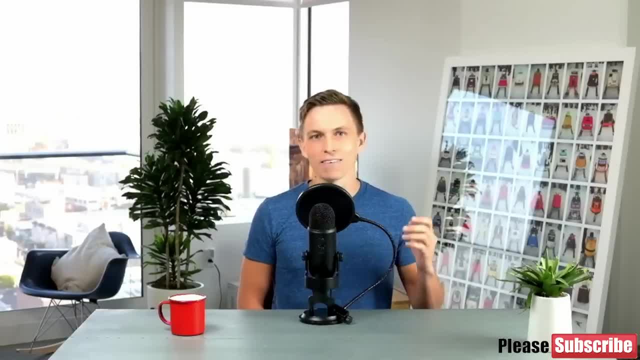 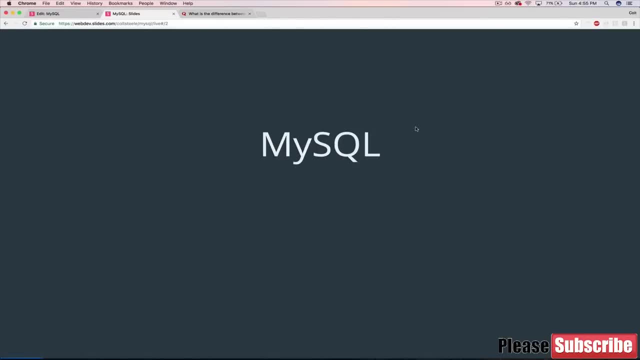 Still it's something. So by the end of the section we'll be doing that. All right, let's get going. All right. so we're going to start off by taking a bit of a step back and talking about two very high level general questions that are pretty central to everything. 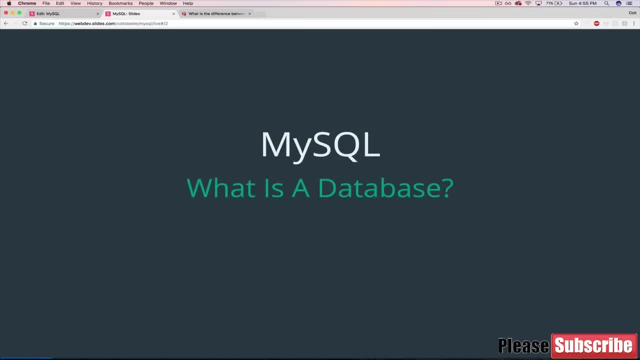 this course is about, And they are: first off, what is database? Seems like it's a pretty straightforward question, but there is a little bit of terminology we need to discuss. And then, secondly, why do they matter? So let's start off with the first question. 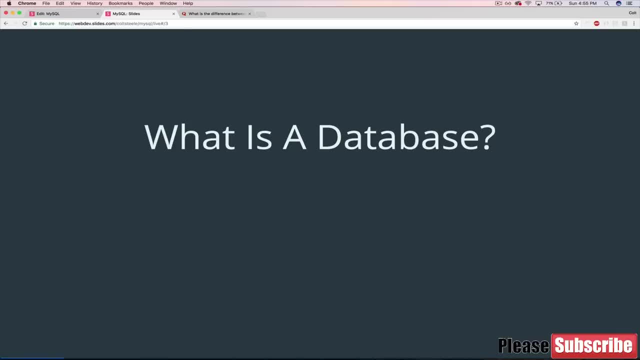 First one: what is a database? What actually makes something database? And there are a couple of definitions that we could go with here. I kind of synthesized some of them into my own definition that has two parts, And the first part is that it's a collection of data, which seems pretty. 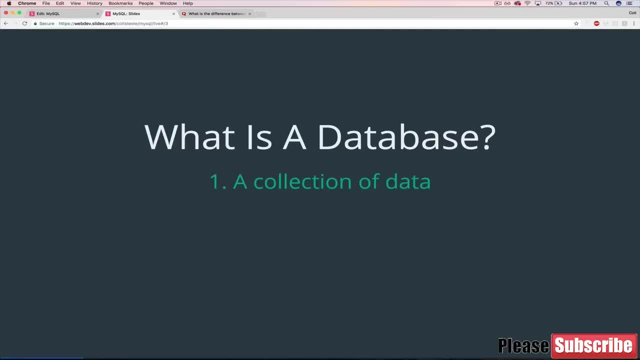 straightforward. There are all sorts of collections of data around us in the real world, things like when you go to your doctor's office and there's a filing cabinet full of medical records, Or even just a to-do list or a list of things to buy at the grocery store. 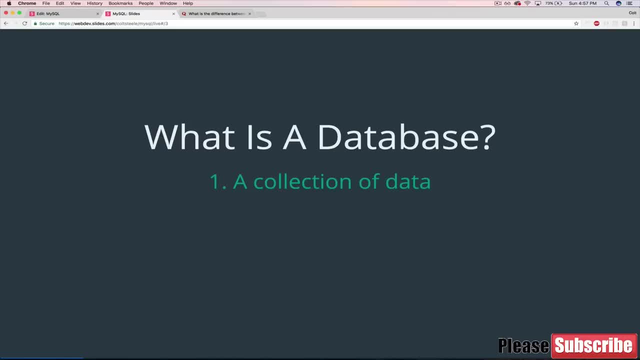 qualifies as a collection of data. Or, going back a little bit in time, if you remember what Rolodexes were, a Rolodex full of different people's contact information that qualifies as a database under this definition, Speaking of archaic technology. 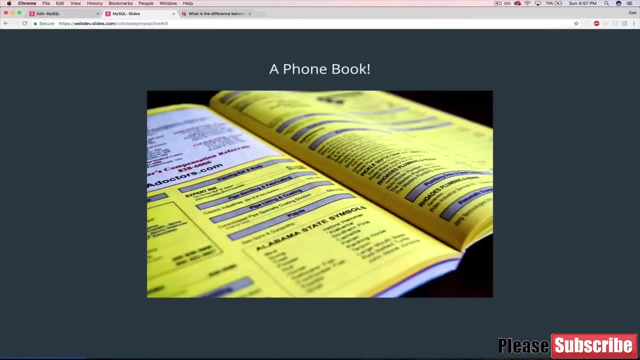 like a Rolodex. another example of a database is a phone book. So I say this mainly jokingly, but I actually have some siblings who don't know what a phone book is or they've never seen one or used one before. It's a gigantic book, basically, that lets you look up people's phone numbers. 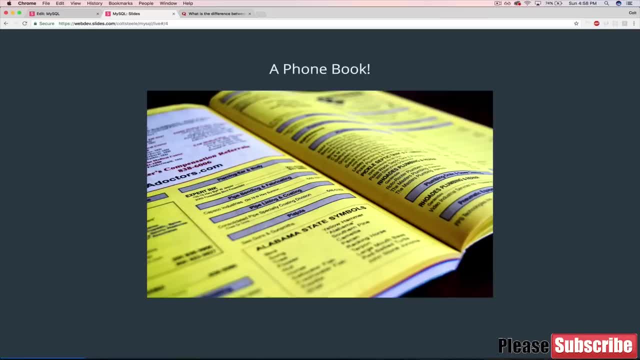 based off of their name. So it's usually organized by last name alphabetically for people. So you would flip through the book until you find someone's last name and then you would try and match their first name and then you find their phone number. So let's take a quick example. 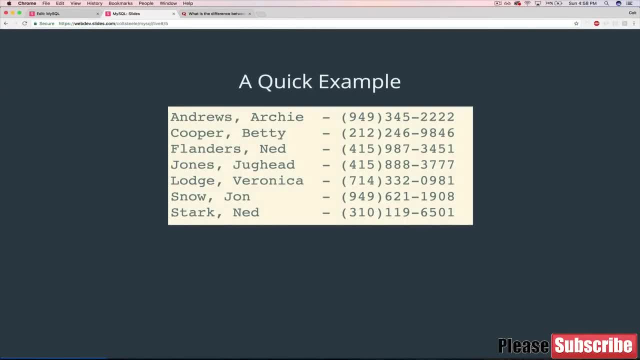 here. This is a fictional phone book. Think of it as just a little section of a phone book. that's a book that has tens of thousands of entries And these are fictional characters alphabetically organized by their last name. So Archie Andrews comes before Betty Cooper, who comes before. 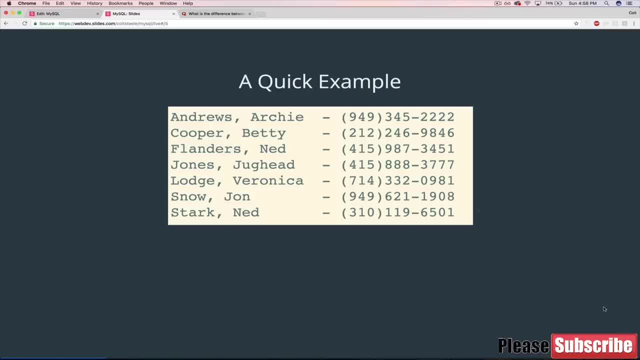 Ned Flanders and so on, And then we have corresponding phone numbers. So imagine you have a gigantic phone book with this information in it and I asked you to do something like find Ned Flanders' phone number. Well, it's actually pretty straightforward. 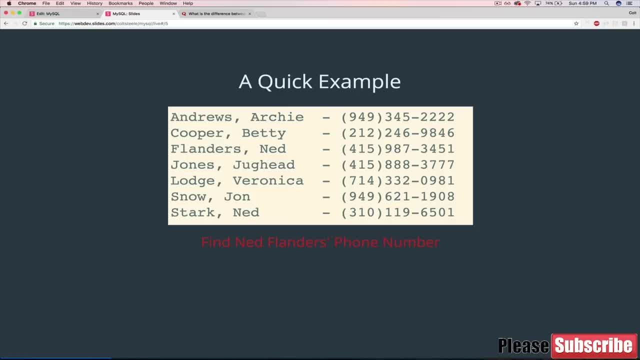 as long as you're comfortable using the alphabet in alphabetical order. You flip through the book until you find F, FL and so on until you find Ned Flanders, and then you find his phone number. It's what the phone book is made for. However, it gets a little trickier, or a lot. 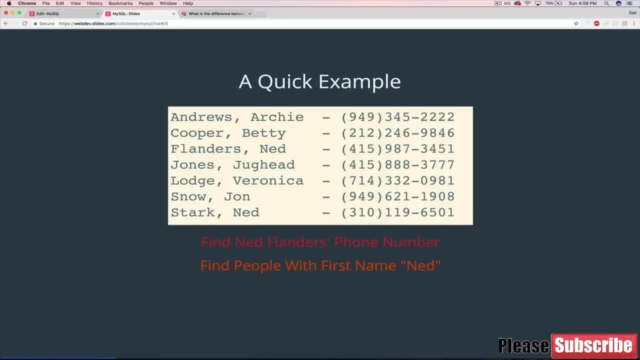 trickier really, if I asked you to do something like find everyone in the phone book who has the first name Ned, There isn't an easy way to do this. You basically would have to go through every entry in the book and check for however many thousands there are. Is this person's name Ned? 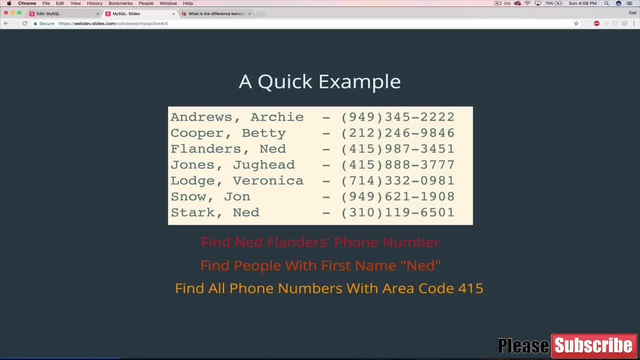 So I have a couple other questions that are similarly difficult. So the point here is just if you were to find all phone numbers with a particular area code, or to find all people who have a three-letter first name, it's not easy and it would take a lot of time, like a ton of. 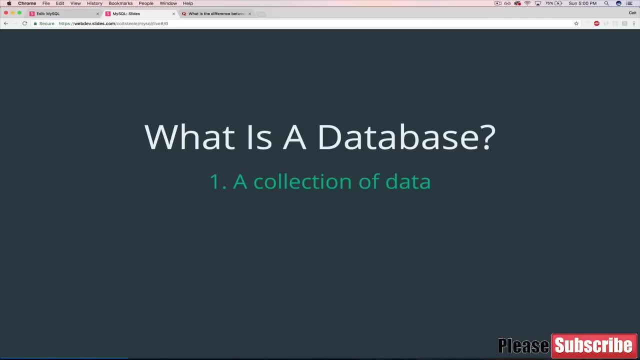 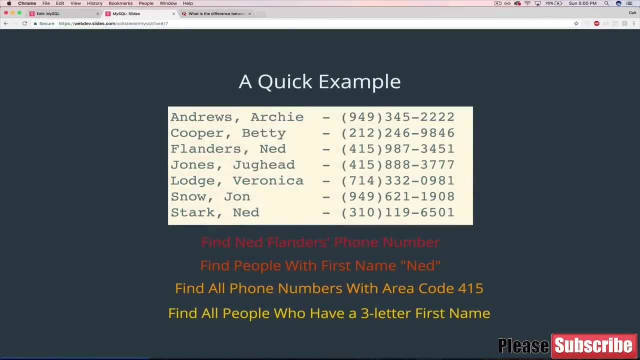 time. So that brings me to the next component of the definition of what makes something a database, in my opinion, which is not just a collection of data. it also contains a method for accessing and manipulating that data. So, going back to this phone book, we would want a way, some sort of 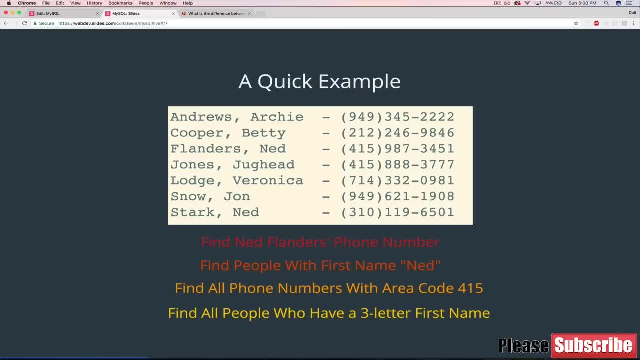 program or code that would allow us to do things like find everybody with the first name Ned, or find all people who have a three-letter first name, or even do things like add a new person into the phone book or change area codes or change phone numbers, or get crazy and just delete. 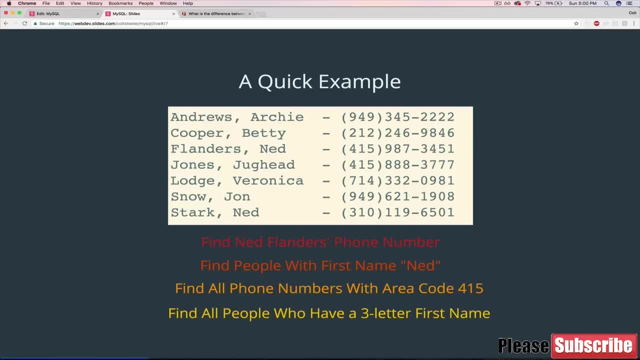 people from our phone book or delete everybody. if we wanted to, We would have some sort of program or part of our database that would help with that. that would allow us to interface with the data. So I did say we were going to dive a little bit into jargon and terminology. I usually try and 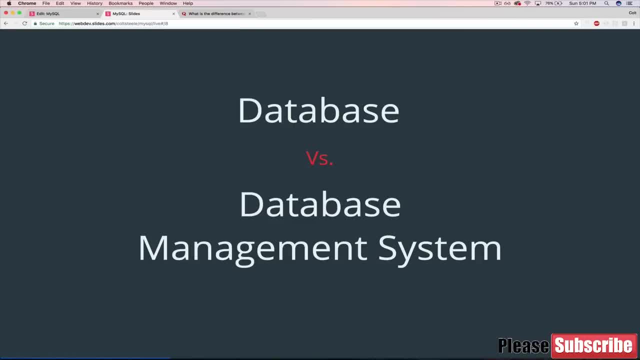 stay away from that early on. Well, I try and stay away from that in general, but especially early on in a course. Basically, if you've read about databases, if you've used one before, if you've read a blog post about them, you may have come across the term database management system or 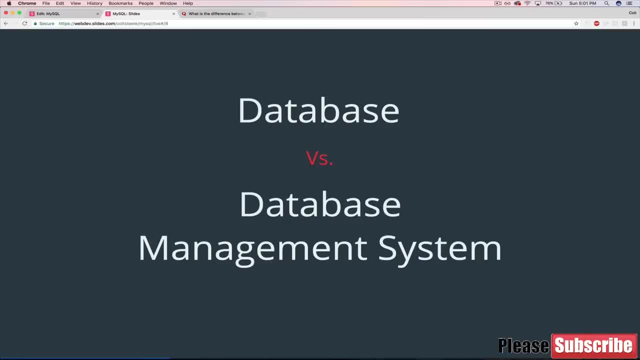 relational database management system, or DMS or RBDMS, all these different acronyms. Basically this right here, what I have on the screen- database versus database management system- refers to the fact that what I just talked about having data, a collection of data- 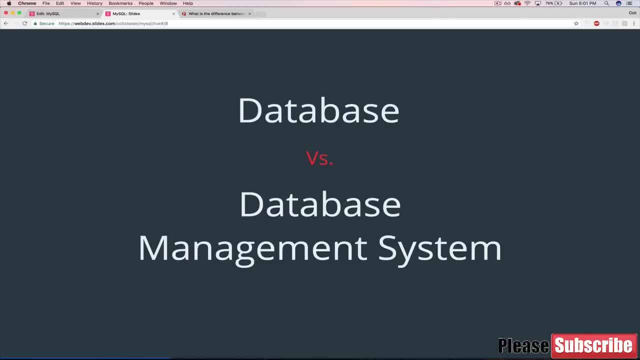 and then having an interface for that data are two different things. So let me show you a quick example. Imagine that you have an application- Let's say it is a dating app- And then you have a database and you're storing all sorts of information. 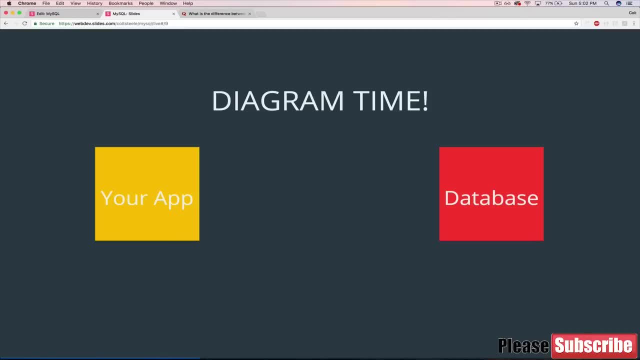 all the different users, all the different messages that have been sent, the photos, whatever else goes into your dating app, But on its own, the database here is basically like our phone book. It's a gigantic collection of data, which is great for storing data, but it really 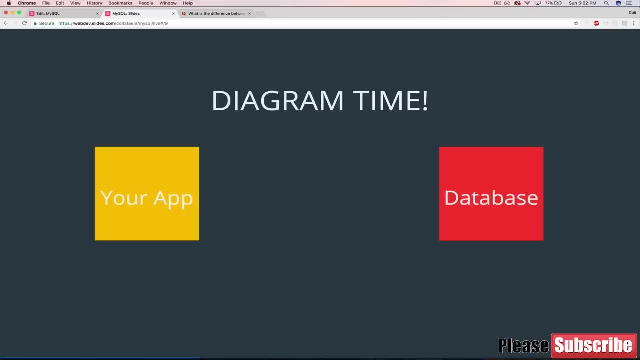 doesn't let us do very much. You can almost think of it as if it was a gigantic file on your computer. So for our application to be able to do things like update somebody's username in the database or edit their profile photo or delete a user if they want to leave our application, 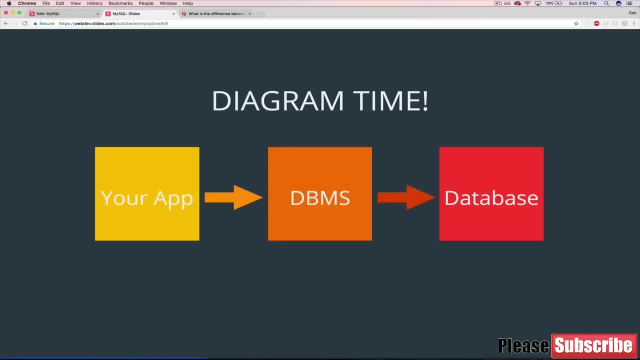 whatever it is, there's a database management system that allows us to interface with that database. So it's just the code or the program that does the talking to our database for us. So we talk to our database management system and it talks to the database. 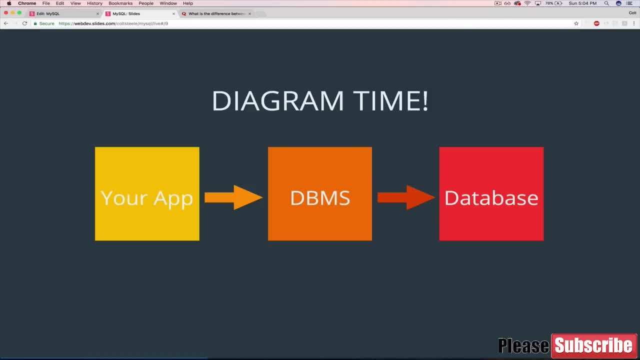 Okay, so for the, For the most part, we're out of the weeds with the jargon here. The reason I brought this up, though, is that oftentimes, when people talk about a database, you actually hear them referring to both of these things- the database management system and the database together- just as a 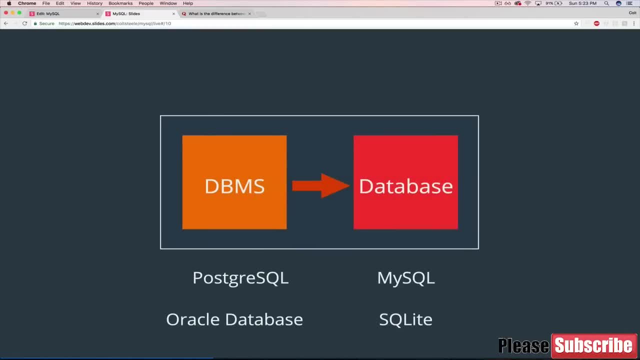 database. So what I have right here is a list of some of the more common databases you'll run into, And actually I just did it there. what I was just talking about, These four things- Postgres, MySQL, Oracle, SQLite- they're not technically databases, They're actually database management. 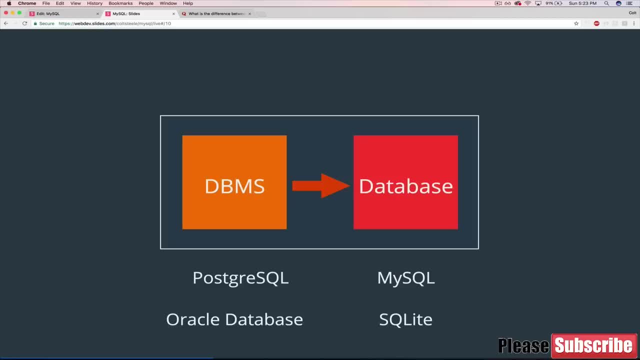 systems, But for the most part people just call them databases. So when we say things like MySQL is one of the most commonly used databases, it's actually one of the most commonly used database management systems. So it's not the end of the world if you forget about that, But it is. 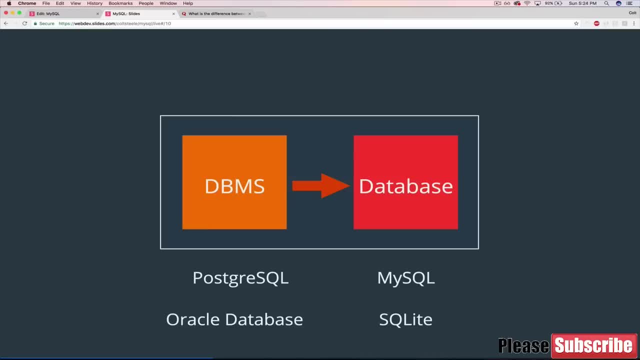 important because it will help you understand later on when we actually start talking about SQL, when we start talking about some of the code that you write to interact with the database. I think it will help you understand what you're doing and that you're giving commands to this database management system, which then 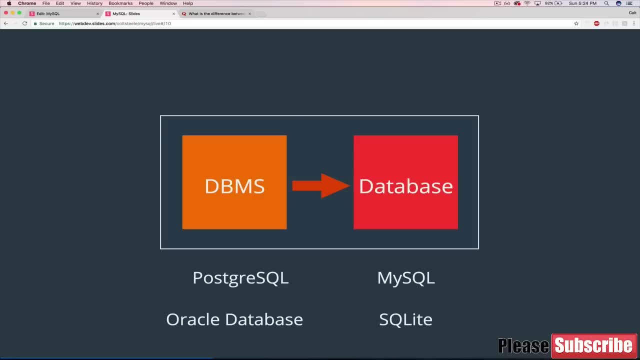 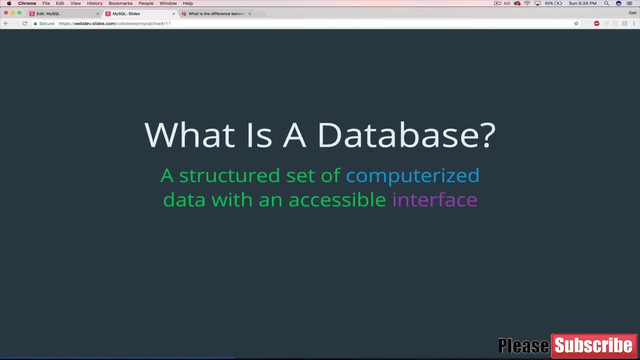 goes and gives commands to the actual data itself or to the database itself. Okay, So to wrap everything up, here's a little bit of a synthesized definition. What is a database? Well, it's a structured set of computerized data with an accessible interface. So in this video we're 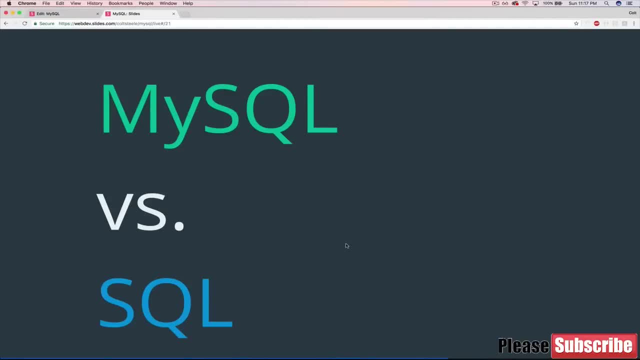 going to talk about one of the more common questions that comes up early on, which is: what is the difference between MySQL and SQL? Or I usually just say SQL, But what's the difference between these two? Obviously, SQL is contained in the name of MySQL. What's the significance of that? So, 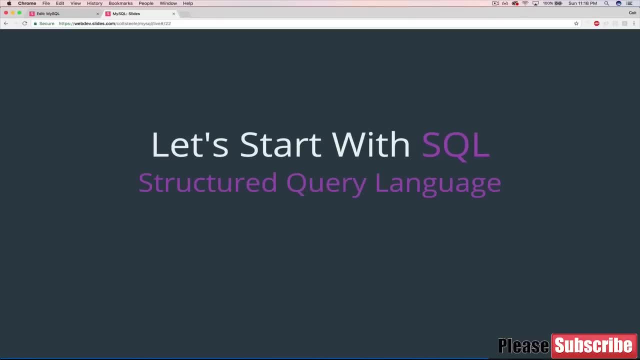 let's start off with discussing SQL, which stands for Structured Query Language. So SQL is the language we use when we talk to our databases. It's the way that we interact and access the data, update data, delete things and basically manipulate the data in our databases. It's the 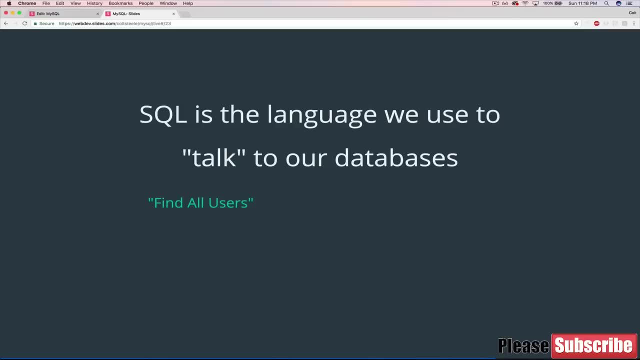 language we use, So it's how we do things like find all users. Now, what I'm showing you here is not actual SQL code. You'll see that in just a second. These are just humanized versions. Find all users who are 18 years old. 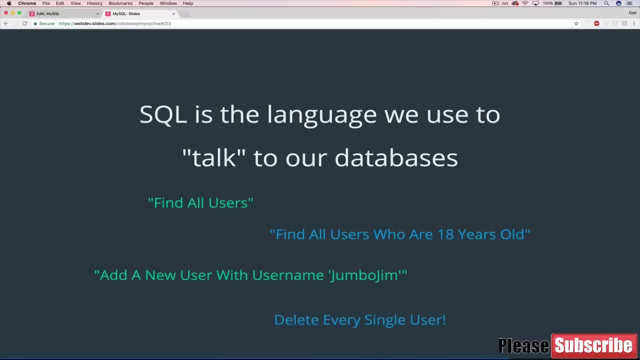 Add a new user with username Jumbo Jim, Or, if we want to get crazy, delete every single user. So these are the sort of things that we use SQL to do. So we write these lines, which are called queries, Structured Query Language, And once we hit enter or once we run that SQL code, 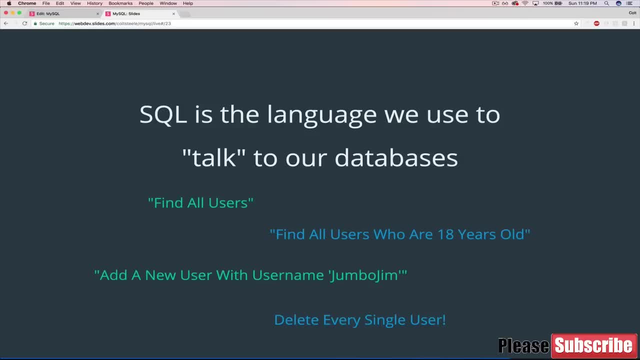 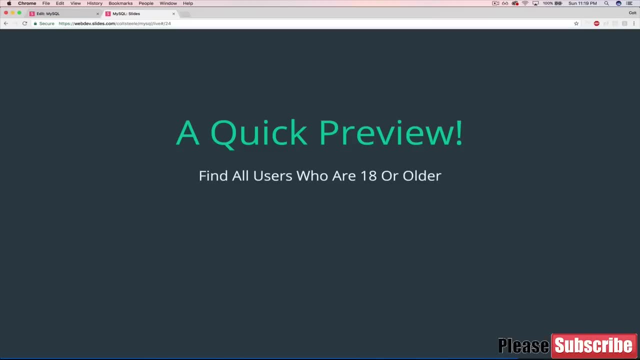 it's executed and it goes off and it talks to our database and it does it for us. So if you are curious of what it looks like, here's a really quick one-line preview. The English version find all users who are 18 or older is translated into this. Select star from. 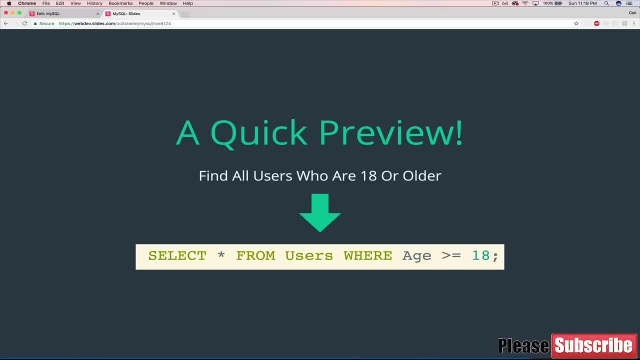 users where age is greater than or equal to 18 semicolon, So hopefully that actually seems pretty straightforward. Now we are going to dive into SQL all throughout this course. You don't need to worry about this exact statement. What's important, though, is that you can see there is. 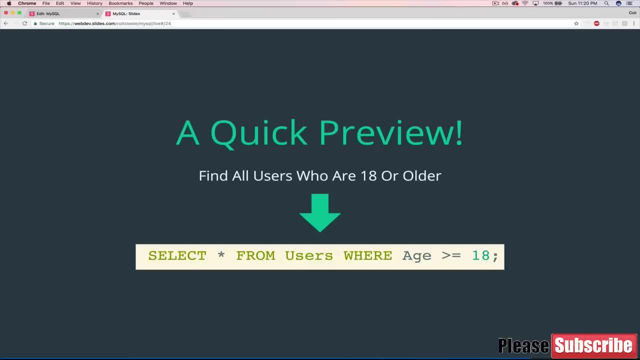 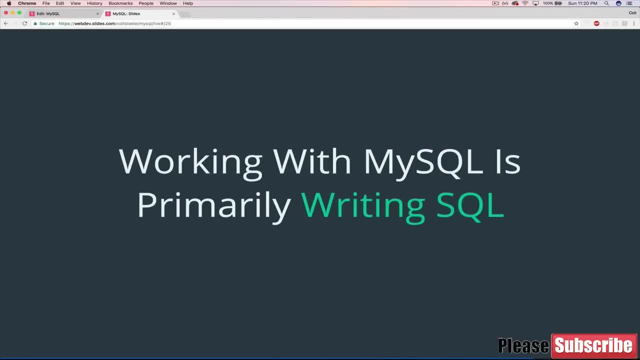 a special syntax we use And that this query here is going to be sent off to interact with the database somewhere. So the next point I want to make is that when we work with MySQL, we're actually writing SQL all the time. So MySQL is what we talked about earlier. 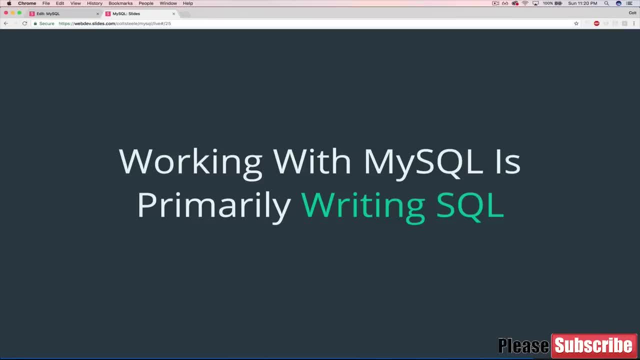 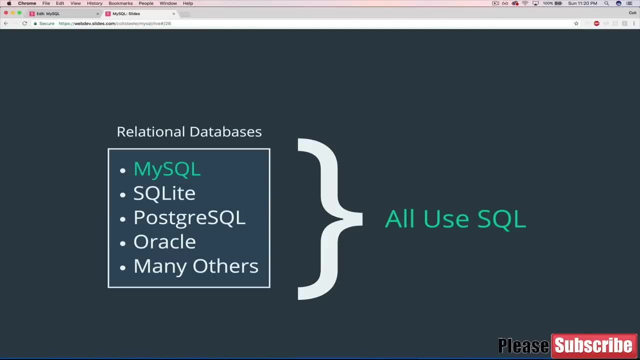 a database management system, and there's a bunch of them out there. Here's some common ones: Postgres, SQLite, Oracle. There's hundreds of others And there's dozens of popular ones, but hundreds of them are all data-based, So I'm going to go ahead and do that. 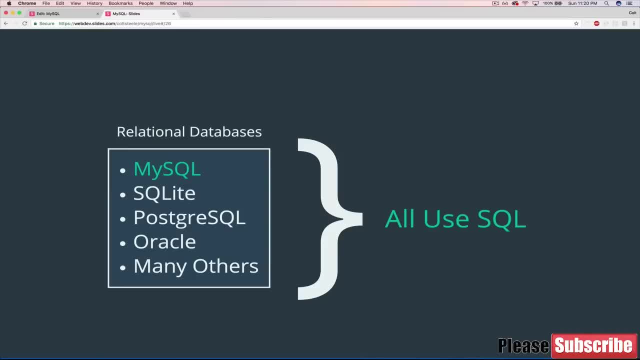 all over the world that maybe aren't as popular. So all of these ones here that I've highlighted use SQL or SQL. That doesn't mean every database ever does, but what are called relational databases do, and we'll talk more about that later when we discuss tables. But for now, the point I want to. 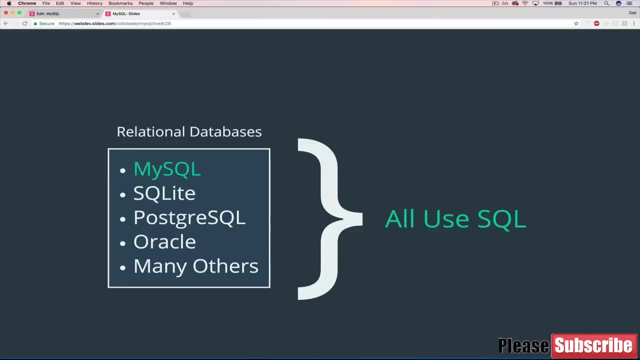 make is that SQL is not unique to MySQL or to Postgres. That's why they all have this SQL in their name. They share this language. So structured query language, SQL, is a standard, basically that these relational database management systems like MySQL implement. So it's kind of a lot of jargon. 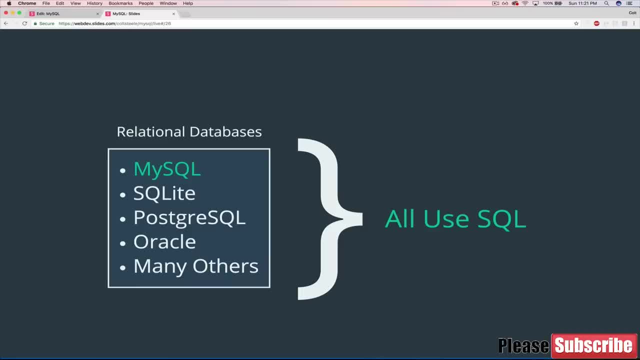 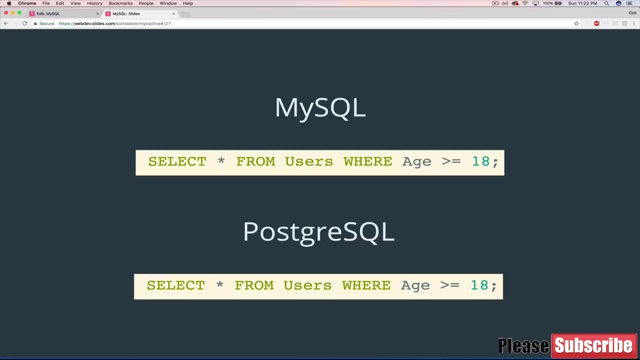 and terminology again, but the main takeaway is that when we use something like MySQL, we'll actually be writing SQL all the time. So here's an example of what a line of SQL code looks like to do the exact same thing In a MySQL database and a Postgres database. here's the MySQL and here's the Postgres, And hopefully you. 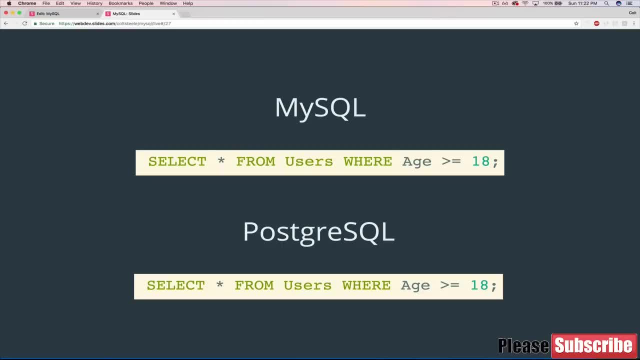 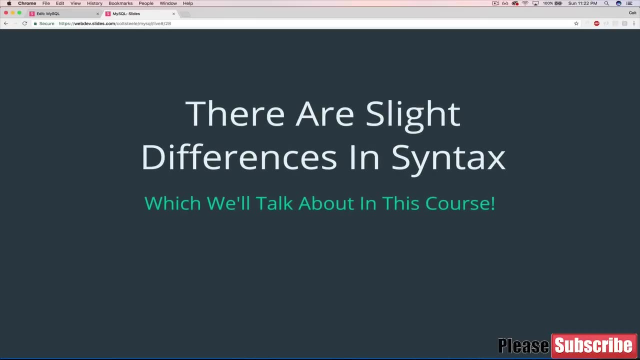 notice. they are identical. Both of these are different database management systems. They have differences to them, but they both use SQL. You will be writing SQL when you interact with these databases. So just to hit that home. there are slight differences in the syntax. They are not. 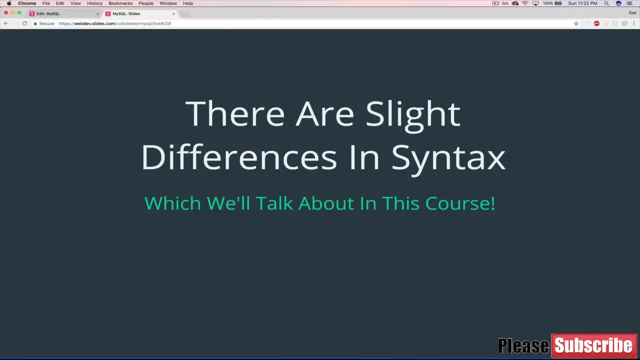 identical, But they're very, very similar. Oh, and I better not forget to mention the SQL standard. So the way that this whole thing works is that there is a standard for how SQL should work. It's actually written down, You can. 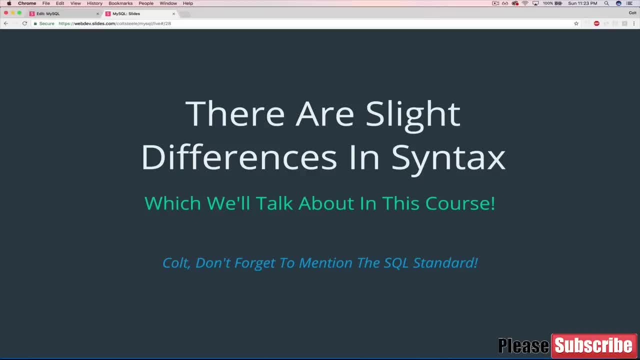 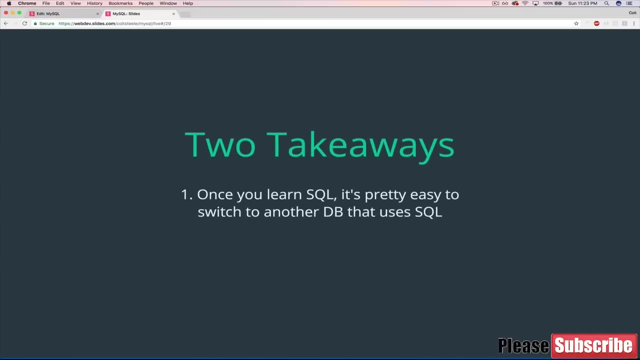 read it online. And all these different database management systems basically, are tasked with implementing that standard in their own database and making it work, And they deviate sometimes a little bit, but for the most part they're very, very similar. So the two takeaways here: One is that once you learn SQL, it's really not that hard to switch to another. 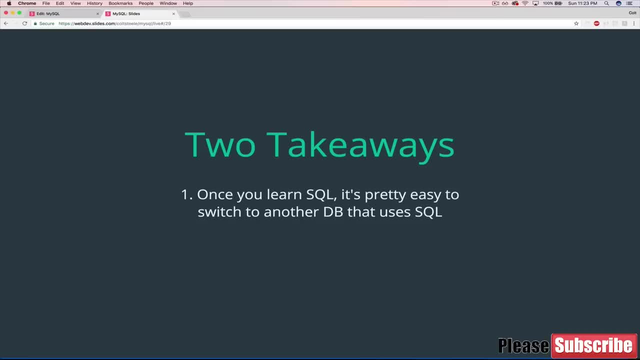 database that also uses SQL, So you're learning MySQL. you could pretty easily switch to Postgres or to SQLite with not a lot of time needed to get up to speed. And the second thing is that what makes databases or database management systems to be specific, what makes them unique? 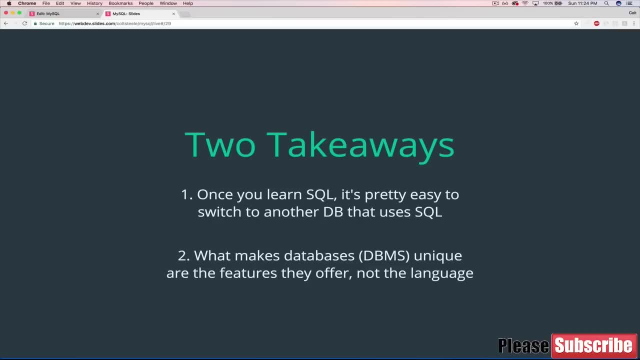 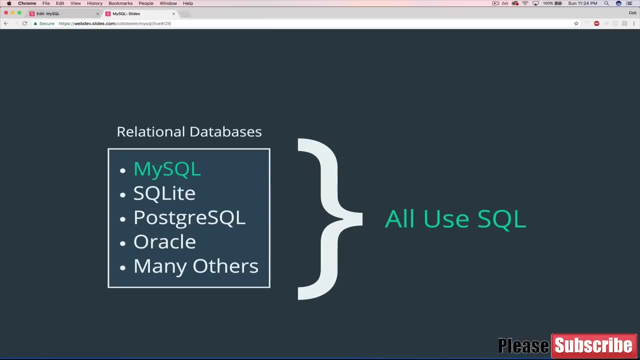 They're the features that they offer, not the SQL or the language itself. So, if we go back to this diagram, all of these use SQL, but that doesn't mean that they're identical. And, yes, you might write the same line of code to do the same thing. 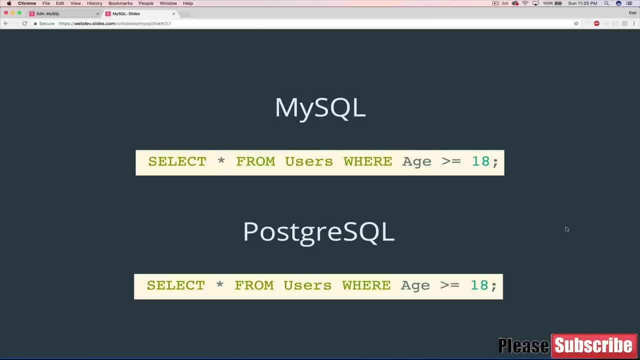 here. So what makes these different are the features that they implement. Things like how secure is one versus the other, How fast is it, How much, how big is the download, How do user permissions work? And on and on, and on. 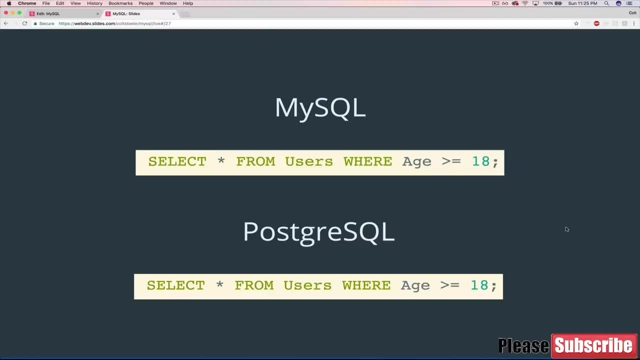 And we'll talk more about what those differences are when we get to a point where they actually make a little bit more sense. I don't want to just talk to you, Okay. so this was about MySQL versus SQL. SQL is structured query language. it exists. 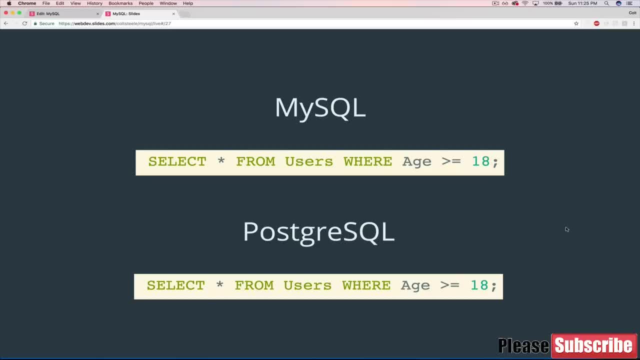 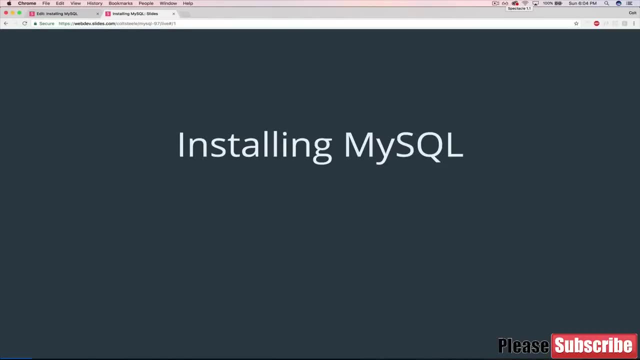 separately from MySQL, And MySQL is a database management system that implements SQL. Alrighty, so we've spent a healthy amount of time talking about the higher level things, kind of setting the stage for this course. Why should you care about databases? What are databases? What's MySQL? Where's that fit in? What's SQL? And so on. 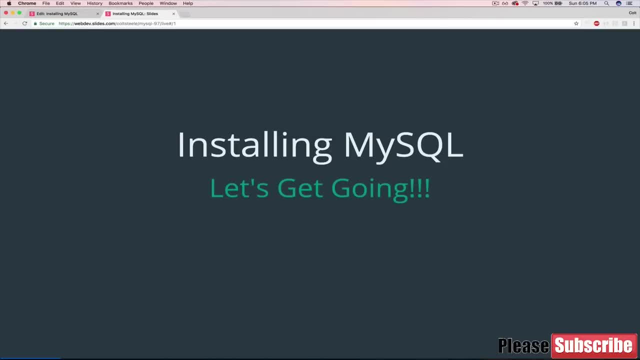 Now it's actually time for us to really get going, So hopefully that's a little bit exciting. Unfortunately, the first thing we have to do is install the tools, install MySQL on your computers. So I want to add a note really early on, which is that in my 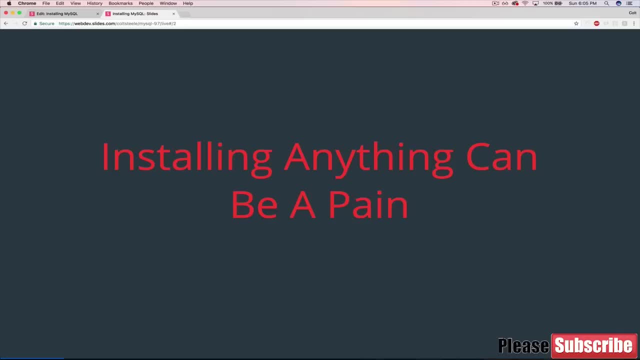 experience. installing anything can be a pain, And that's true for someone who is an experienced developer all the way down to a complete beginner. It's always a potential point of friction where things can go wrong, And nothing is more frustrating than being excited to do something, being excited to learn something new and then have it. 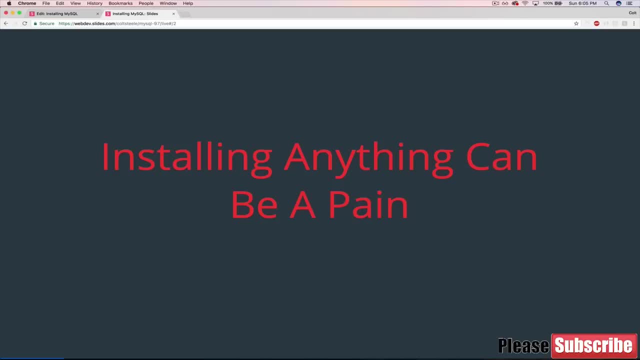 not work Or have to spend hours trying to figure out why it's not installed correctly and what's going on. In my opinion, it's one of the worst parts of being a developer And then also in my experience teaching, I've seen a lot of people get discouraged. 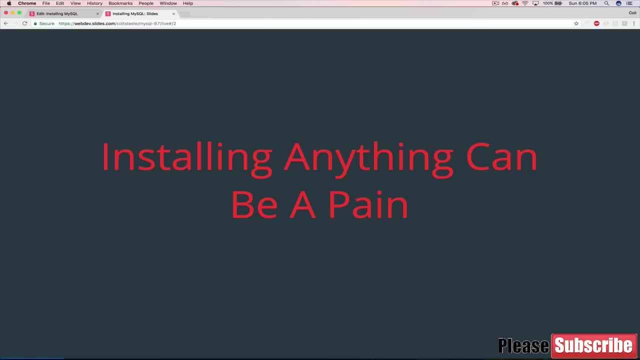 really quickly when something doesn't work out. If you're unable to to install MySQL when you want to learn MySQL, it might just send you in a different direction and you might end up learning another database like SQLite that doesn't require as much setup and 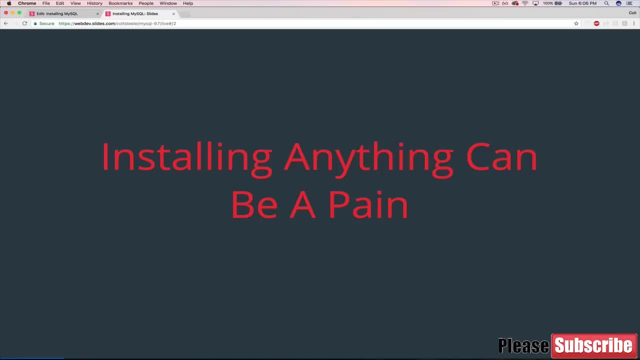 that's easier to install, So we don't want that to happen. Nothing against SQLite, but this is not a course on SQLite, So I just wanted to put that out there. that keep in mind. installing can be a pain, but I'm going to do my best to try and make it painless. So we have three options. 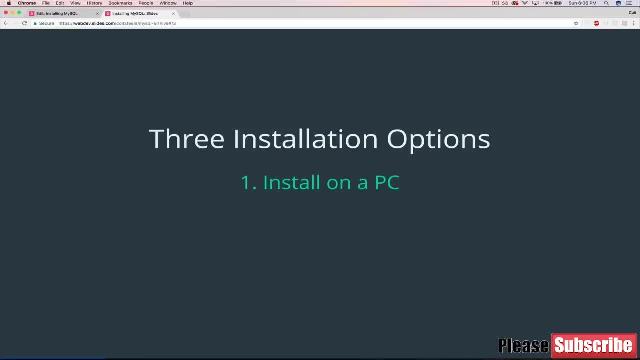 The first one for installation is to install it on a PC. So if you have a PC, if you're a Windows user, you can follow those instructions. The next option- you probably guessed- is that you can install it on a Mac. So if you're following along using a Mac, this would be a good choice for you. 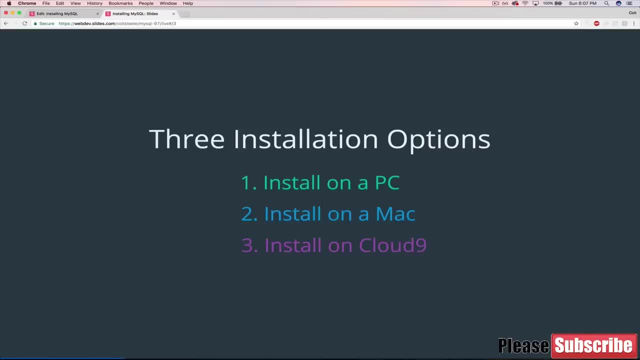 But there's also a third option, which is to install it using a service called Cloud9. So if you've taken my other course, you may be familiar with Cloud9. It's basically an online interactive development environment. In just a couple of videos I'll go. 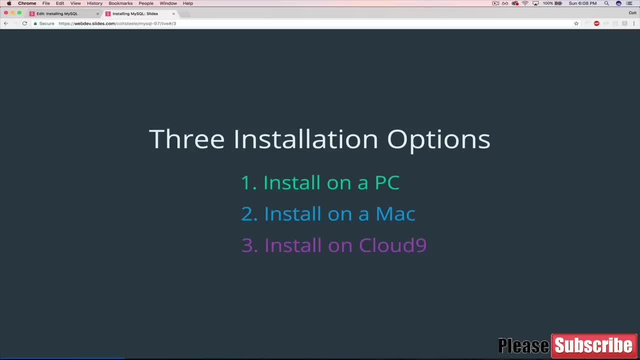 into some more detail about it And, before we go any further, I just want to highlight that installing using Cloud9 is, without a doubt, the best and easiest way to get started, And it's what I recommend that you use, which is why I spent so much time drawing this little box around it. 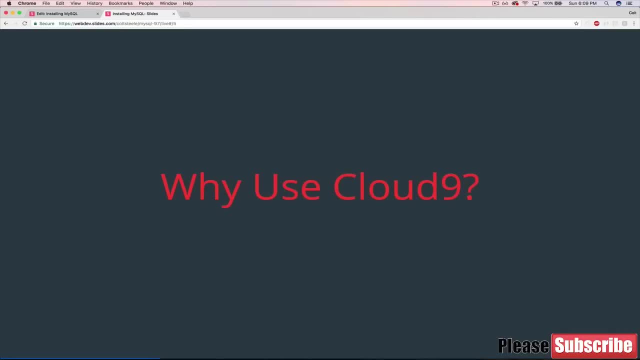 install on Cloud9.. So why is that? Why do I recommend that you use Cloud9?? There's a couple reasons. The first is that it's what I'll be using in the course. So, rather than doing everything on a Mac and confusing the Windows people, or doing everything on a PC and confusing people on a Mac, 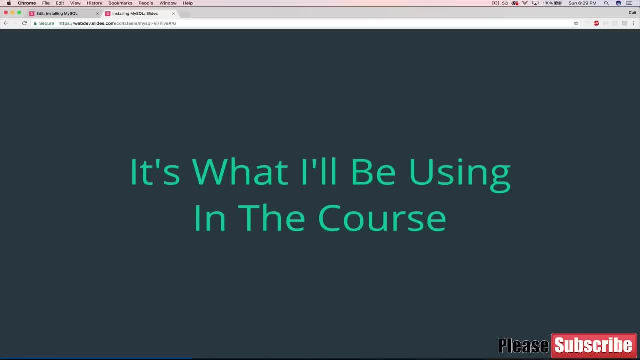 I'm going to use Cloud9,, which is something that anybody can use, regardless of the type of machine that you own, how old it is, how much RAM you have, what operating system, that doesn't matter. It levels the playing field. So, because I'll be using it in the course, I think it makes it a lot. 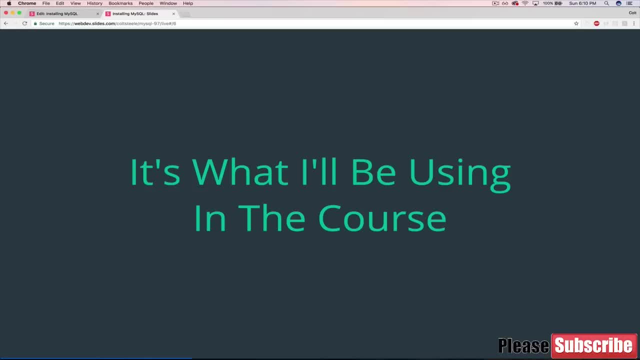 easier. So if you're someone who's pretty confident as a developer, of course, feel free to install it however you'd like, But I highly highly recommend that you use Cloud9, at least early on, because you'll be able to follow along much, much easier. And the second reason, equally important, is that 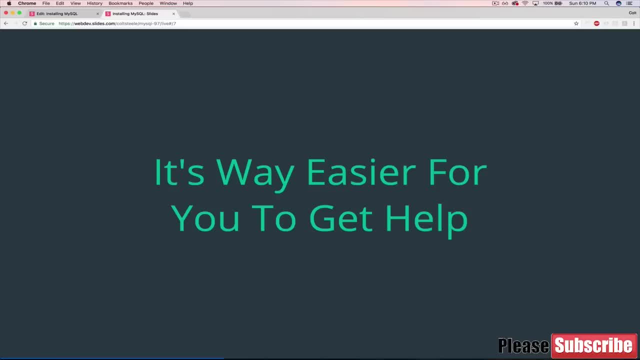 it's way easier for you to get help if something goes wrong. If you're doing a project or an exercise and something doesn't seem to be working the way you expect, or you hit a bug, or you're just not sure what you did wrong, you can easily share a link. 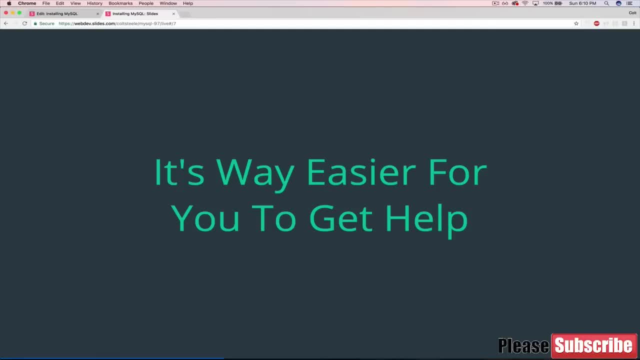 to your environment through Cloud9 and post that on our discussion boards and either me or one of the TAs can help you out. So it's way easier for you to get help. If you were just working on your PC or Mac and you're trying to explain what's wrong, you're going to have to take some screenshots. 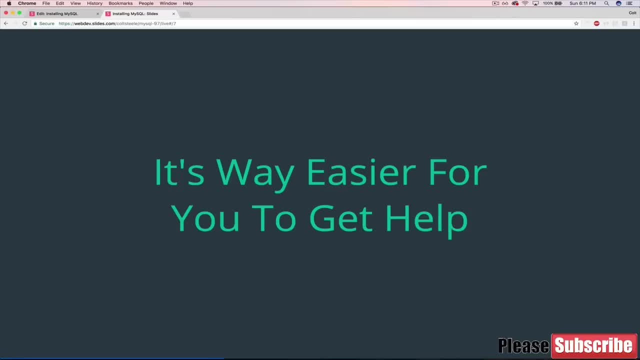 you're going to have to upload them. you might have to copy and paste some stuff from your terminal, But if you use Cloud9, and I'll show you this when we talk about Cloud9 in more depth- you can just take the link of your workspace and share that and anyone will be able to look at your. 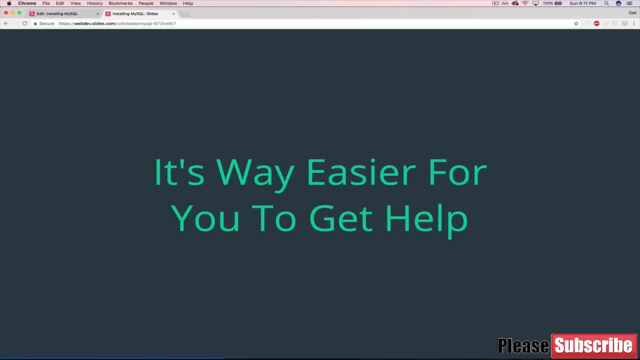 site and diagnose a problem. And the third reason that I didn't write down- and this is a really important one- is that installation is basically painless. You have to sign up for an account, and that's about the worst part. Once you're past that, it's one command to get MySQL working. 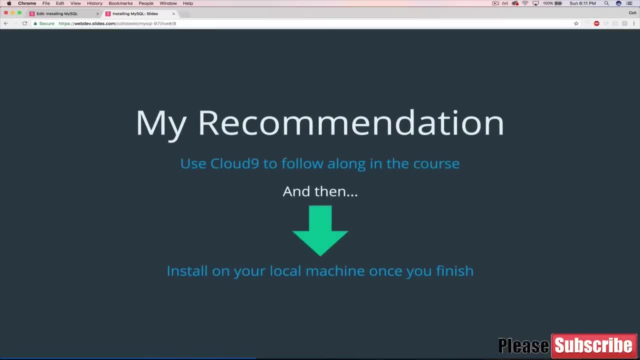 which is pretty amazing. So, with all of that said, this is my recommendation or prescription for how you should go about this course. Use Cloud9 to follow along throughout the course. Everything that I do in Cloud9, you'll be able to replicate yourself in Cloud9.. 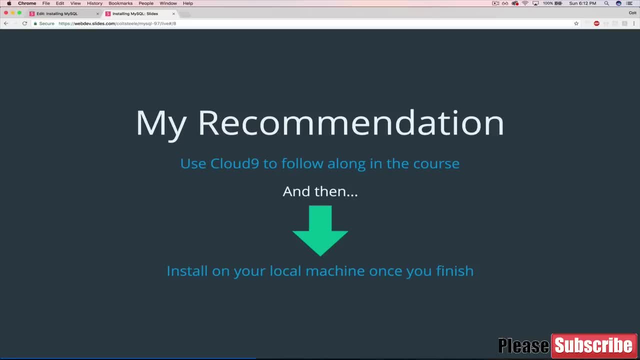 And then, once we've finished the course, you can return back to the installation instructions and then install it on your Mac or your PC natively. I'll talk about what that means. what's the difference between installing natively versus Cloud9 when we talk more? 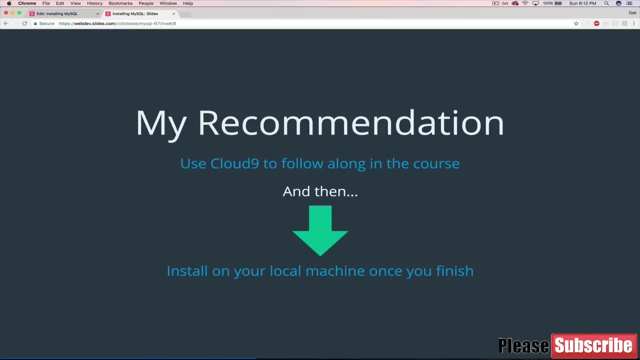 about Cloud9 in just a little bit. So that's my recommendation. I highly highly recommend that you start with Cloud9, and then later on, if you'd like, your PC or your Mac. All right. so enough about that, Let's get down to business, All right. 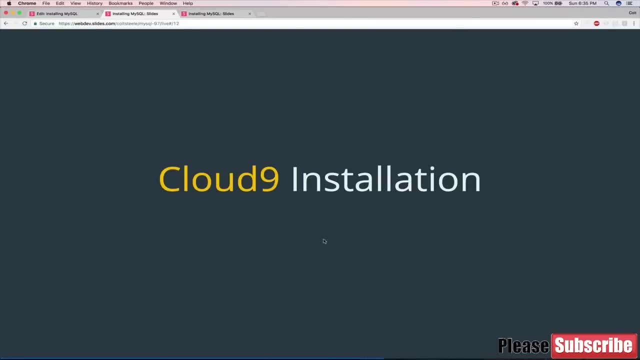 so in this video we're going to go over the specifics of setting up Cloud9.. Now, just to recap, Cloud9 is a cloud-based developer environment, So what that means is that it contains everything you need to create applications and have databases, basically. 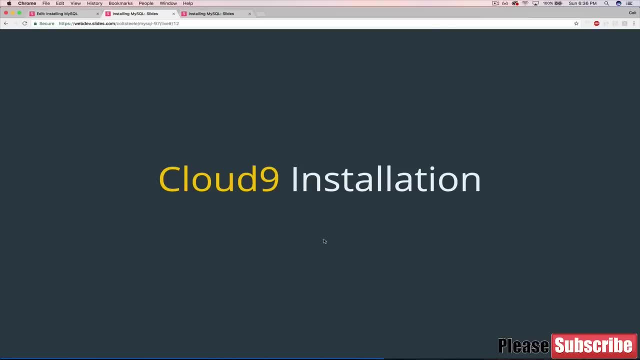 a terminal alongside of a text editor all in one inside of your browser so that you can instantly get- and I know I sound a bit like a marketing show for Cloud9, I promise I'm not. We don't have any sort of deal, I wish we did- But what it lets you do is get something going really quickly and 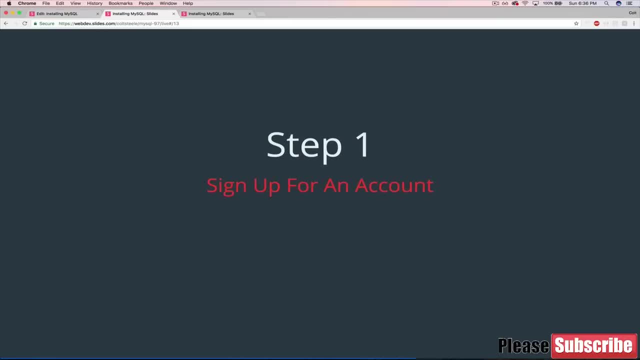 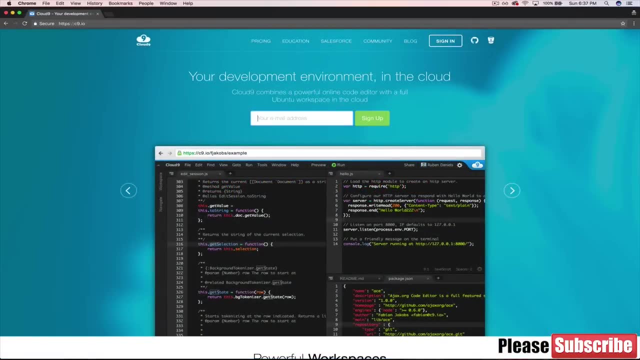 very, very painlessly. So the first step is to sign up for an account. So if you visit the URL c9.io or you click on the link in the description- but it's probably going to take you to the link in the description, but it's probably going to take you- 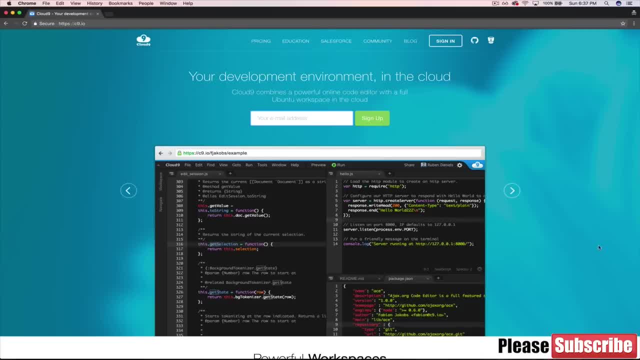 to the link in the description. but it's probably going to take you to the link in the description. pretty short URL: c9.io. you should see this page if it's your first time visiting and you don't already have an account. If you already have an account from another course, you can wait until. 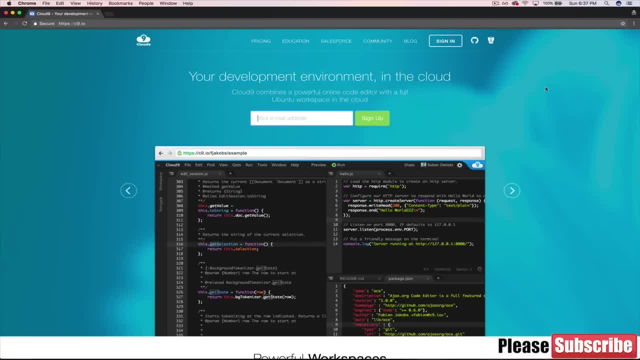 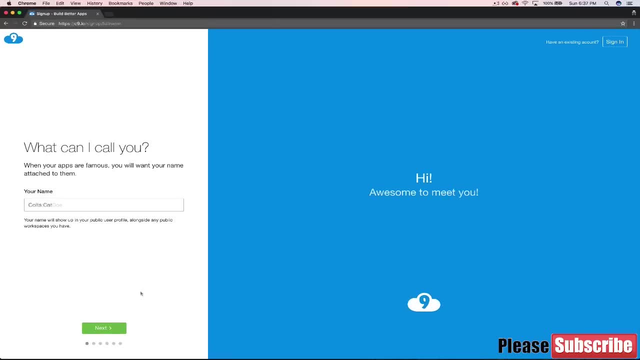 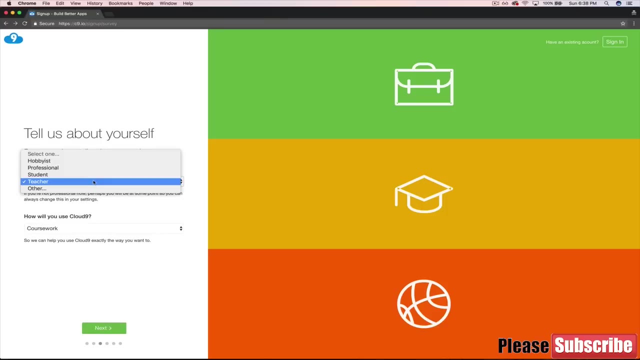 the next step where we create our new workspace. So if you don't have an account, all you have to do is enter your email. hit sign up. you'll have to fill in some information. pick a username. choose the kind of developer that you are. 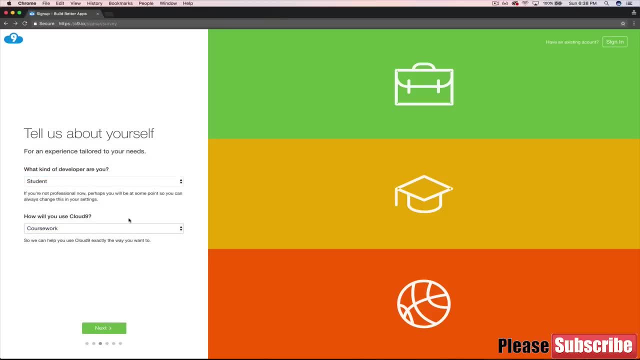 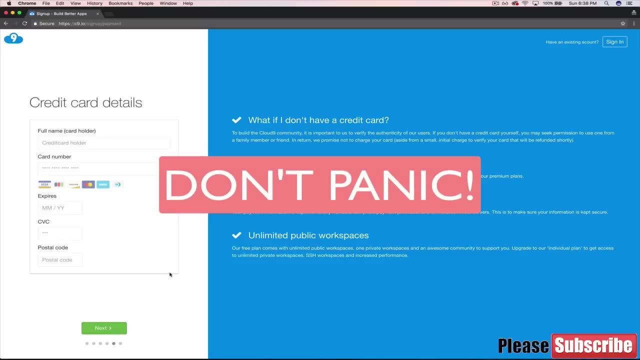 choose how you'll use Cloud9, click next. make sure your details are correct. Now, this is where some people may panic, but don't panic. It asks you for credit card information. Now, if you notice here, it does say that you will not be charged. So there is a perfectly functional free tier of 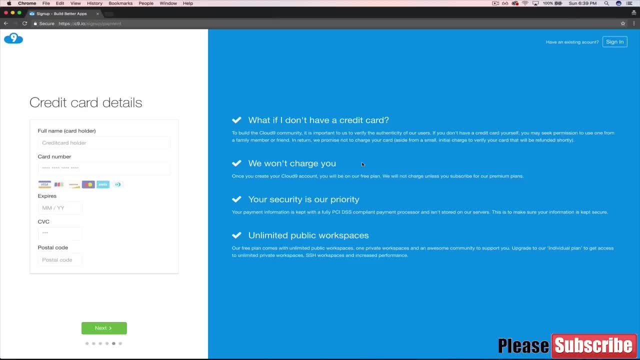 Cloud9,, but you do have to have a credit card to sign up this way. Now, as I said, don't panic, because if you don't have a credit card- which I know a sizable number of my students actually don't have credit cards- You may come from a country. 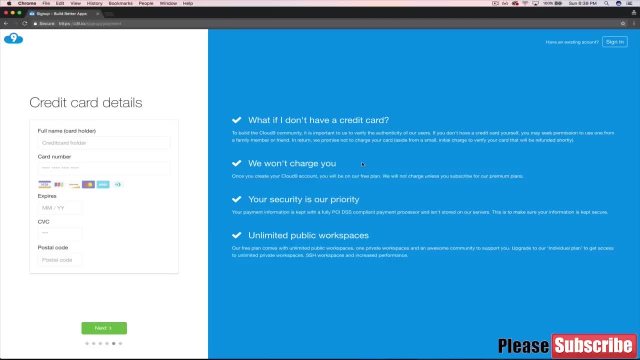 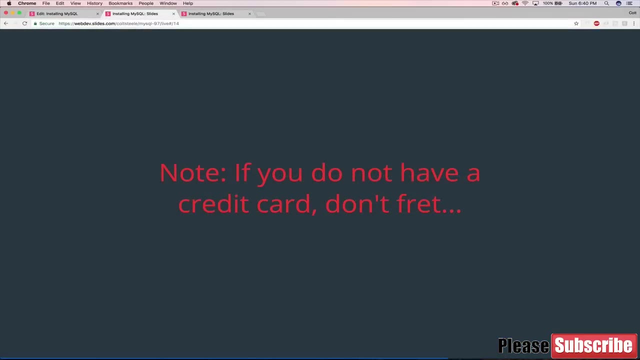 where credit cards aren't as prevalent. You may be too young to have a credit card, or you just may not have one for some other reason, And that's totally fine. It's not a barrier to using Cloud9. It's a little bit of a tiny hurdle, So there is a workaround. So Cloud9 offers educational. 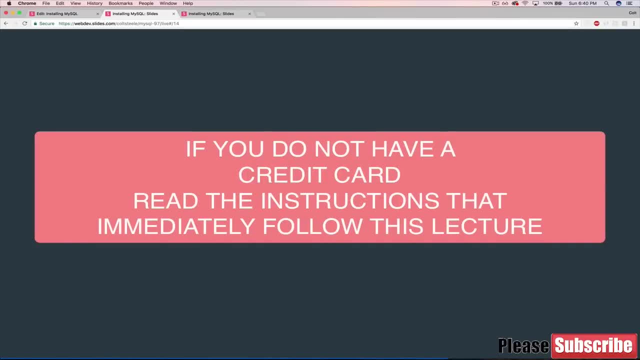 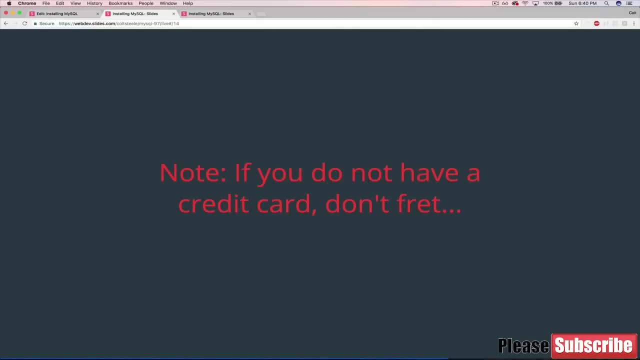 accounts for teachers and instructors, And what that allows me to do, or allows you to do, is to sign up without having to sign up for a credit card. So if you don't have a credit card, you don't need to use a credit card. Now the only problem is that I have to manually add you in. 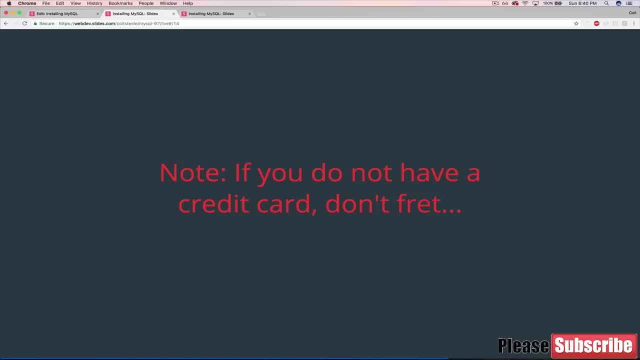 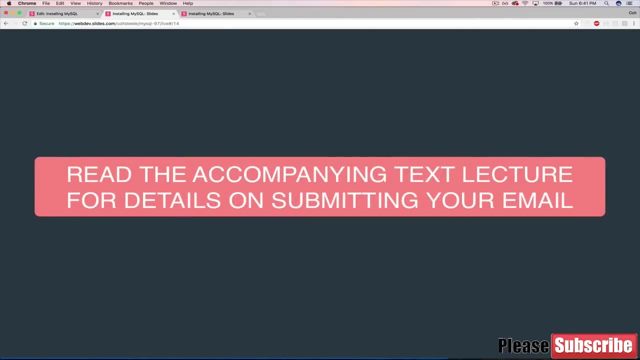 as a student under my educational workspace. So again, it does take a bit more time because either me or one of the TAs will have to manually add you in. but we're committed to doing that. We want to make sure that everyone can follow along, even if you don't have a credit card. Now if you do have, 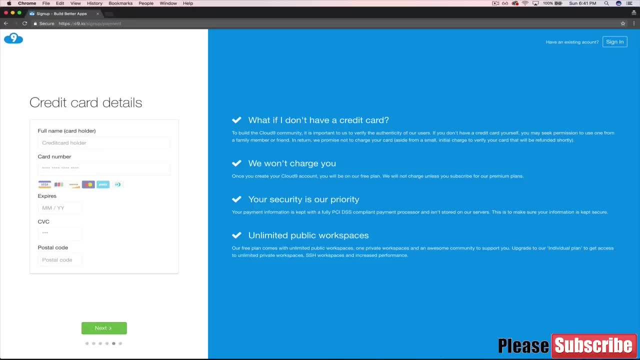 a credit card. I do recommend that you just fill this out, because you will not be charged And it's just going to be faster. You won't have to wait for me to fill this out. So if you do have a credit card, I'll wake up in the morning and check the discussion boards on Udemy. You'll just 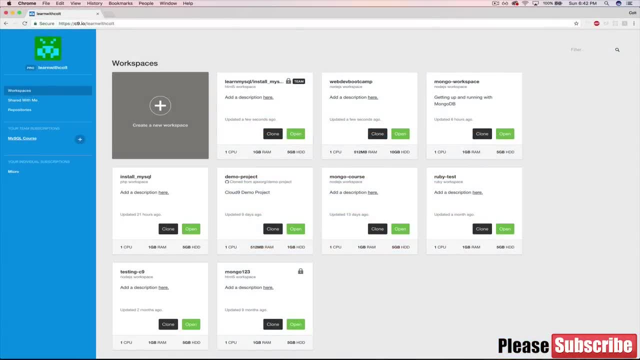 be able to get started right now. So, once you've filled all that information in and completed the signup process, you should see a screen like this. although you won't have any of these workspaces here, So in Cloud9,, when you create a new workspace, what you're actually doing is creating. 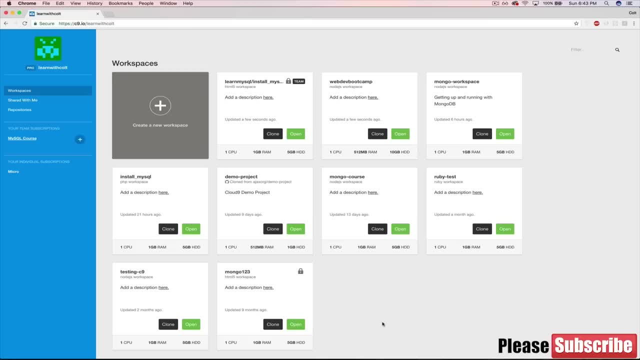 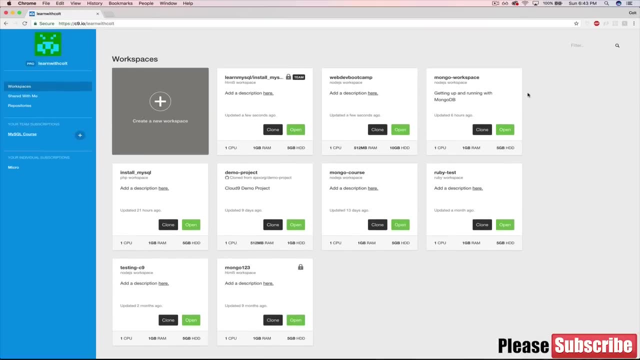 a new developer environment, separate, partitioned off environment that you can work in. So actually you can see, here I have a couple of different environments going. Some of these I use all the time, like the one for my web dev bootcamp course. Some of them are just. here's a test that I made. 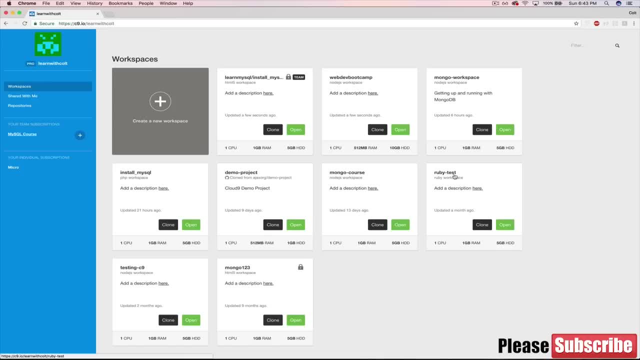 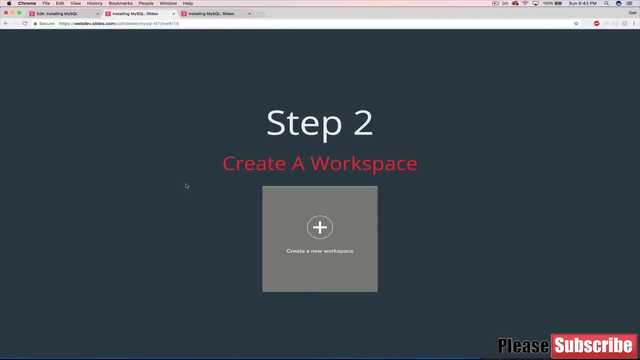 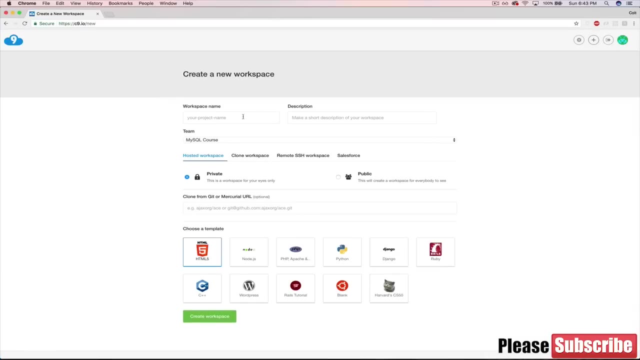 to see how a Ruby environment works in Cloud9.. Or here's one where I installed MySQL, which is what we'll be doing in just a moment. So step two is to actually go ahead and create a workspace. So we click Create a New Workspace And you're welcome to call your workspace whatever you want. I'm. 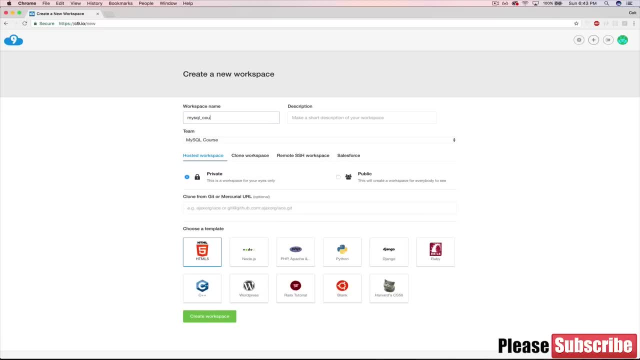 going to call it MySQL underscore course, And then I'll go ahead and set it to be public. It's up to you if you want your work to be private or public, but you don't really need to worry about anybody seeing what you're doing anyways. 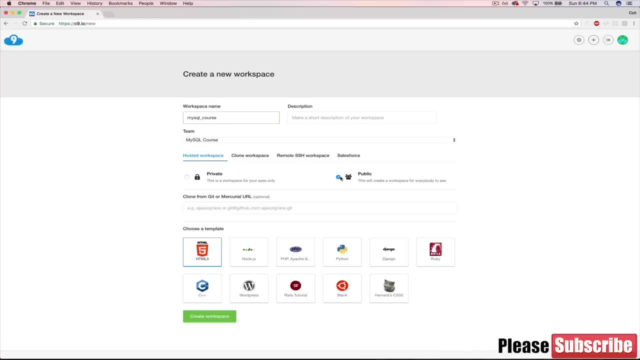 But if you do want to make it private- that is how Cloud9 makes some of their money, But I'm going to make mine public- Then we have these templates down here that we can choose from. So there are these presets that allow us to create a new developer environment really quickly, And 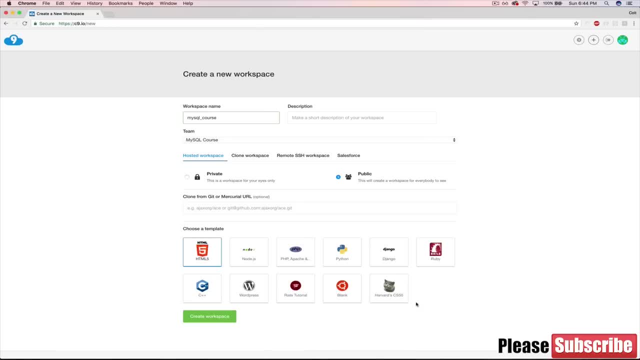 that doesn't really matter for us in this case. So you can pick any of them, but I recommend you just pick HTML5. It's the simplest one. Basically, it's going to be an empty workspace for us, So then we click Create Workspace, We wait a little bit and wait a little. 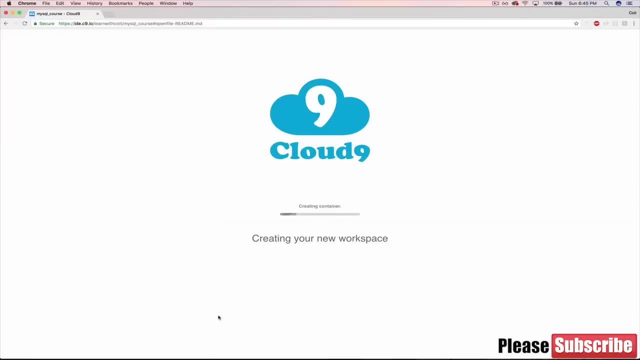 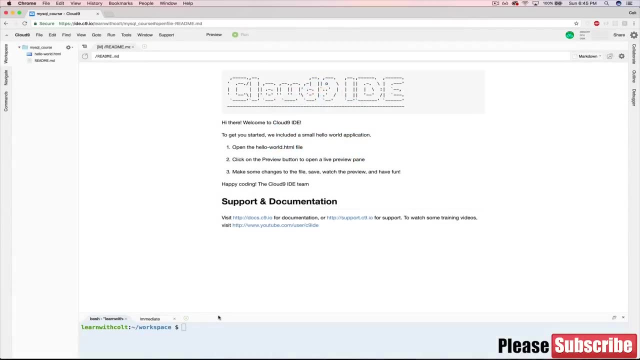 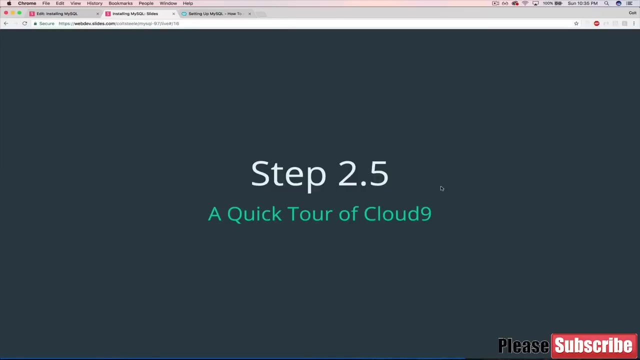 more And finally, once it's done, you should see something like this. So that's it for this video. In the next video, we're going to talk about what this interface means and how we navigate it All. right, Now that we have our workspace set up, the next thing we want to do is take a really quick tour. 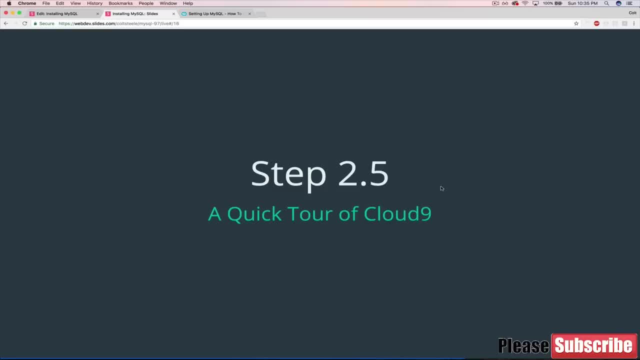 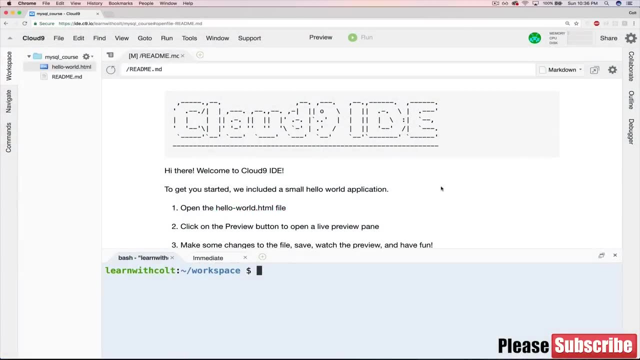 two to three minutes of how the interface for Cloud9 works. So once you've created the workspace, you should see a window that looks something like this: I did increase my font size to make it a little easier for you to read, So yours will probably look a little nicer, but otherwise. 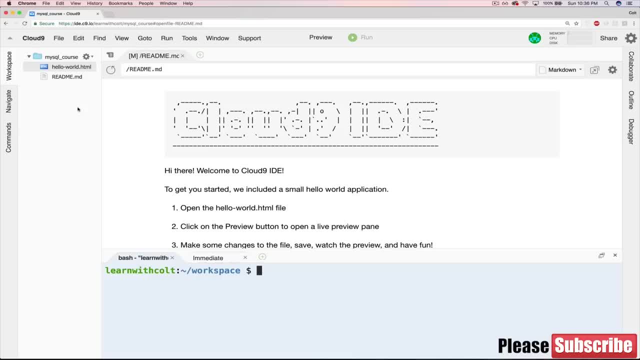 they should look the same. Before we actually dive into the interface, I want to emphasize what actually happened when you created a workspace, because I think it's pretty cool. I mentioned that Cloud9 is a cloud-based developer environment- When you created that workspace, 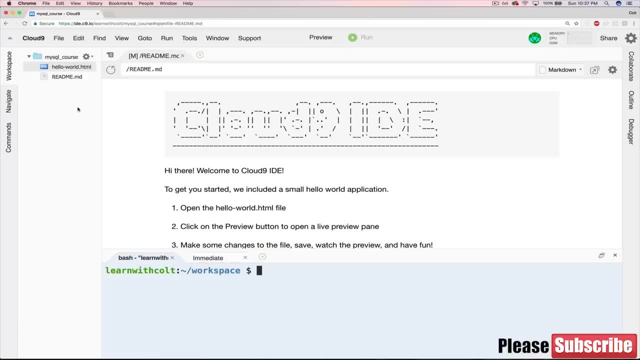 Cloud9 has a computer somewhere, a server that made you a little bit of space just for your little developer environment and basically made you a section on a computer that's private for you. It only holds your stuff, your files, And right now there are only two files in there. 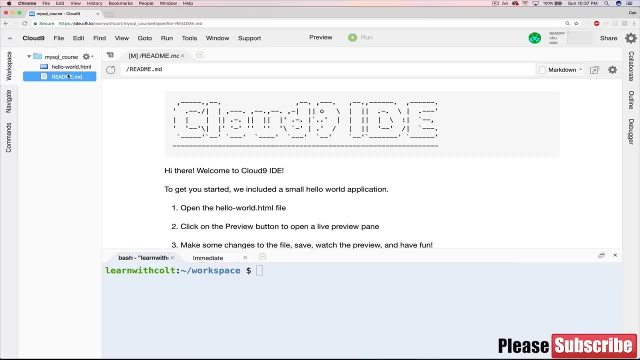 which we can see over here: helloworldhtml and readmemd. Those are both just automatically created. The HTML file is created because we chose that HTML template. If we had chosen a Python, or let's say we chose a Ruby template, we would have a helloworldrb file. But that doesn't really. 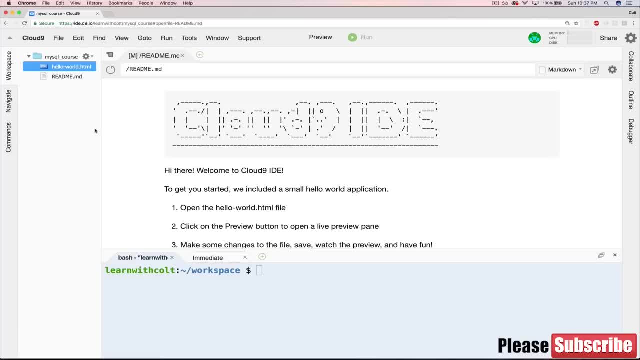 matter, because we're going to get rid of both of them anyway. But the idea is that there is space actually on a computer somewhere that is running all of this. It has these files on it. When we install MySQL and get it running, it's not actually going to be running on your machine or in this. 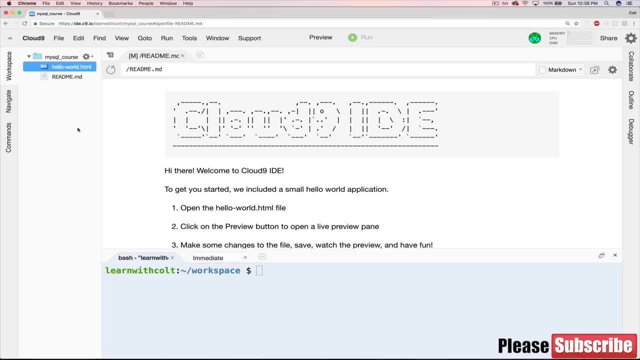 case on my machine. It will be running on Cloud9's machine, And this is just a browser interface for me to talk to that machine, which is pretty amazing when you think about it. So that's enough of that. Now let's take a look at the interface. We have three main sections. 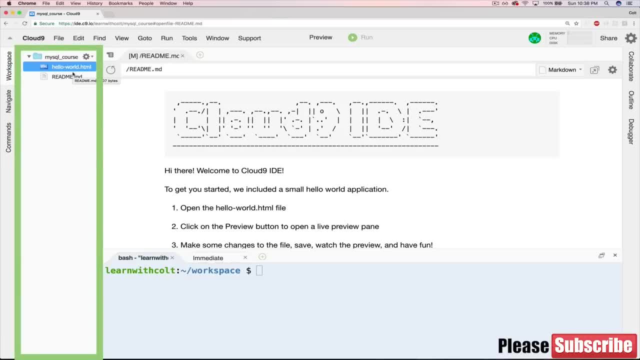 The first one is what I'll call the file tree. It's basically a visual representation of the contents of your workspace. So, as we already talked about, there's two files there. right now. As we create new files and directories or folders in this course, you'll see them pop up over here. The next area I'll call your attention to: 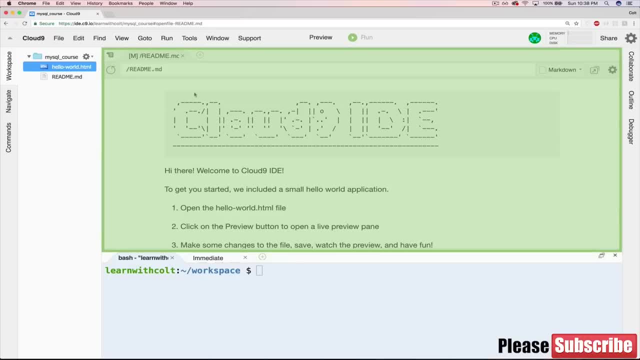 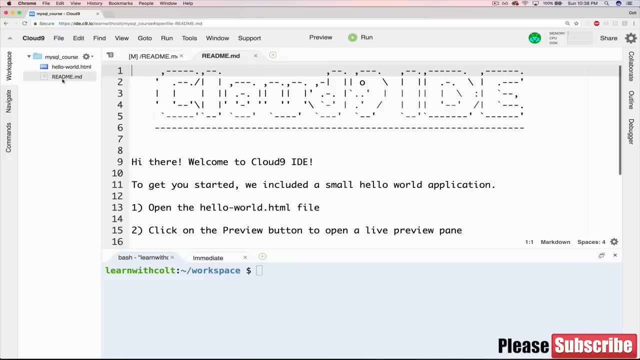 is this middle area. I'll call it the text editor. So if we open up one of these files like readmemd, which is what is currently open, if I double click that, it opens up, as you can see here, readmemd. Don't worry if you've never heard of Markdown. 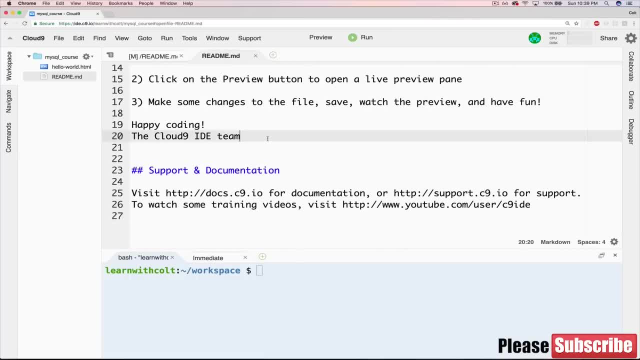 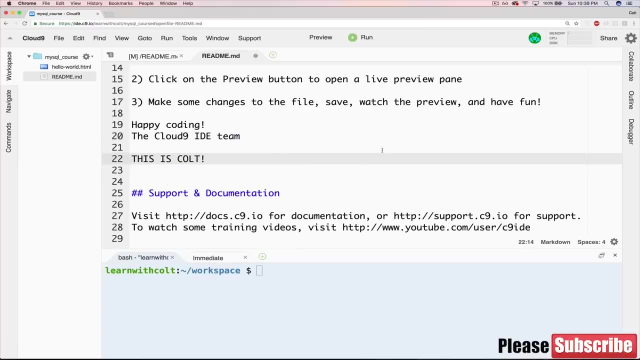 That's not super important at this point, But I can now go in and edit things And if I hit save on Mac, it's Command S On a PC Control S, So I can switch files to the HTML file by double clicking. And now it opens up a tab here I can go back to that other file. 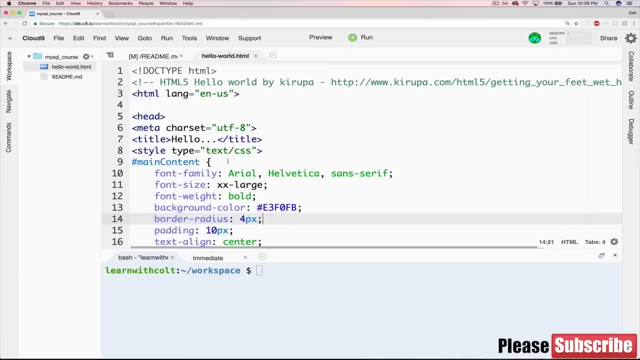 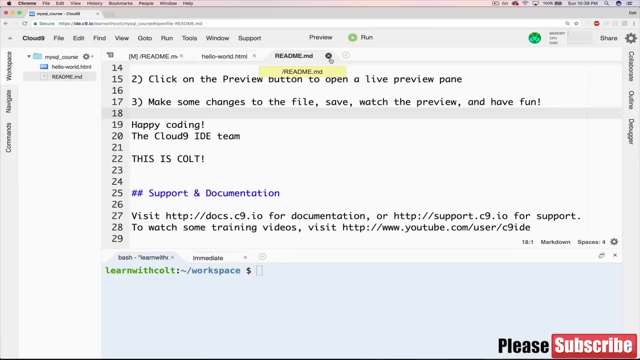 I'll close out of it Now. you don't need to know HTML, of course, for this class, But the point here is that we have files We can double click and we can see them over here. The last thing that I'll show you before we get started is that you can see that we have a lot of files here, And we can see them over here. The last thing that I'll show you before we get started is that you can see that we have a lot of files here And we can see them over here. The last thing that I'll show you before we get started is that you can see that we have a lot of files here And we can. 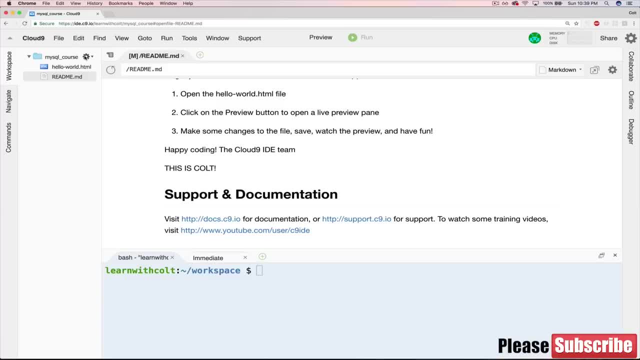 see that we have a lot of files here, And we can see that we have a lot of files here And we can move on to this bottom section is how to make a new folder or a new file. So what you can do is right-click on this space right here And you can scroll down and find new file or new folder. So 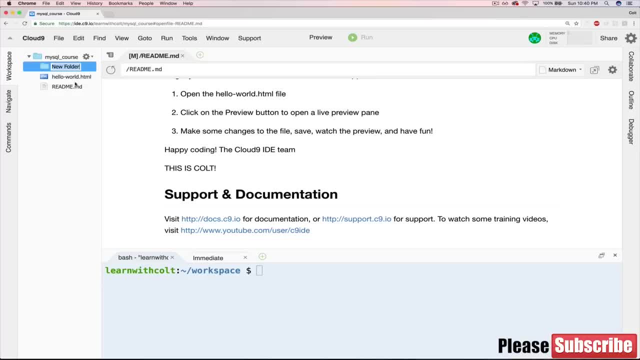 let's make a new folder And I'll just call it testing. Then I can right click again and go to new file. you can also do file new file, just like you were working in a real text editor natively on your computer. But I tend to do this here- new file, and then I can call this whatever. 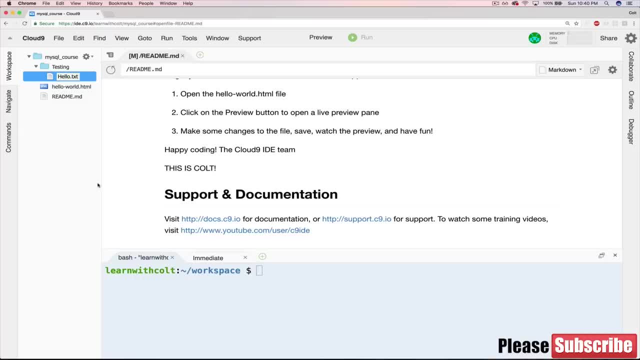 I'll just say Hello and I'll make a txt file. Now to open it I can double click, put whatever I want in there. Now, if I switch, you see that little dot, that means it's not saved. I can go. 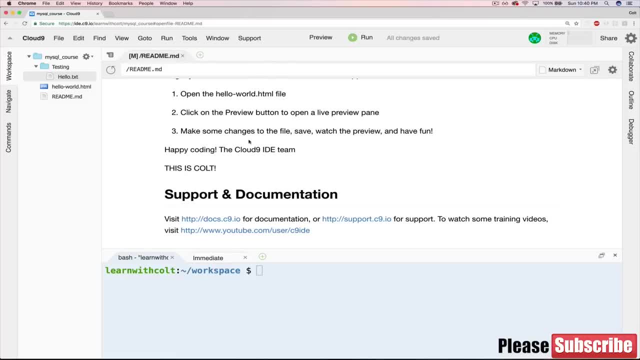 back and save it and close out, And now we have three files over here as well as a new folder. And now we have three files over here as well as a new folder. So that's pretty much all there is to the text editor area And we'll be working with this later. 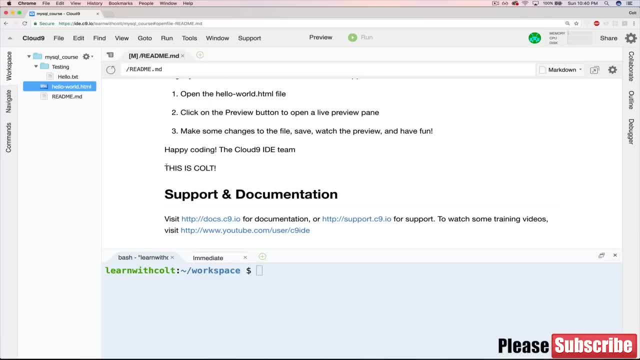 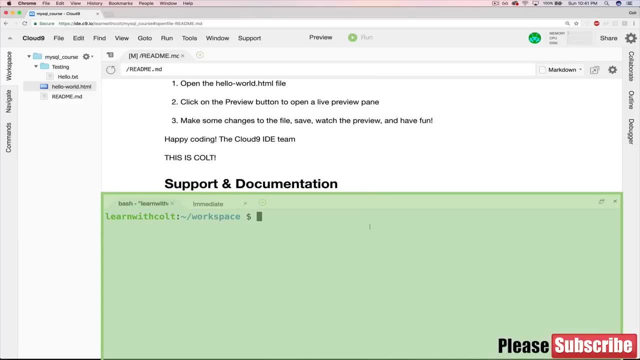 on when we're creating SQL files that we're writing our code in and then running all at once. Then the last section that I'll expand down here is the shell, or the terminal. If you're familiar with any sort of bash shell, this is exactly a bash shell, And if you're not, don't panic. 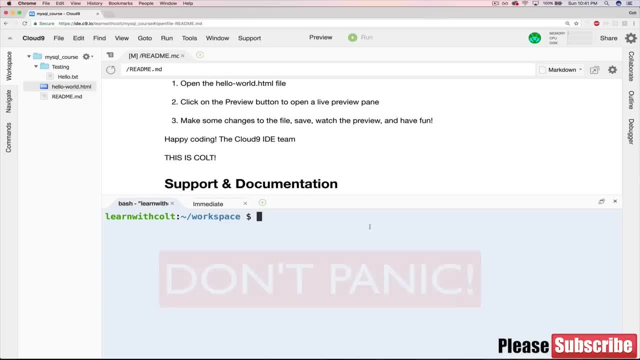 I'll throw up that little don't panic thing again. You don't have to know that for this course, because if you're not familiar with any sort of bash shell, you can just go to the tutorial and you can just throw up that little don't panic thing again. You don't have to know that for this course. 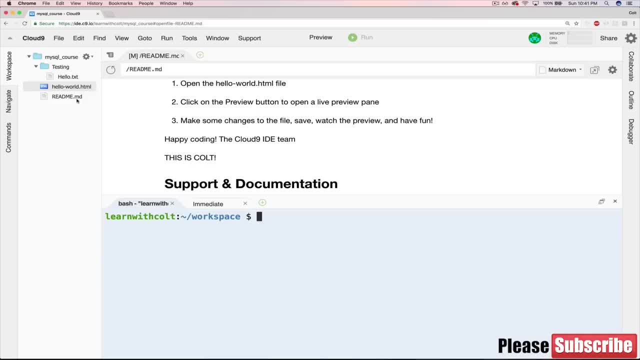 because if you're not familiar with any sort of bash shell, you can just go to the tutorial, and because of the way Cloud9 works, we have this visual interface for navigating our folders and files. But it definitely is not a bad idea to learn some basic terminal commands. I'll include a link. 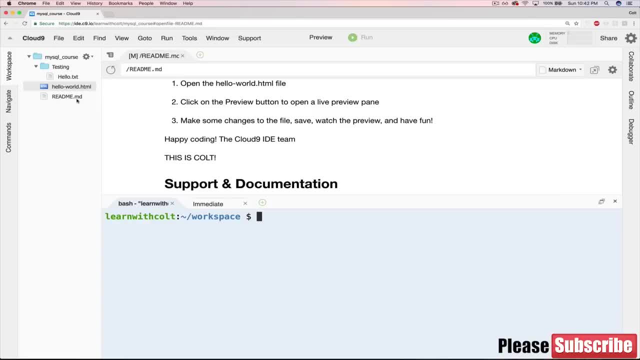 to some of my favorite resources for learning that if you'd like. But again, you do not have to know how to navigate the terminal to do this course. But just to show you that this is a full-fledged terminal. I can do things like ls to list all the files in my current directory And you can see I. 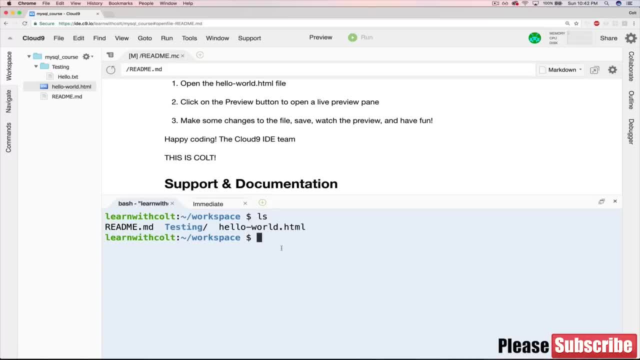 have readme helloworldhtml and testing. I can change directory into testing And now if I type ls I get hellotxt. So I'm inside this directory And I can do things like print working directory. Now we will be running commands from this terminal, mainly to initialize MySQL as well as 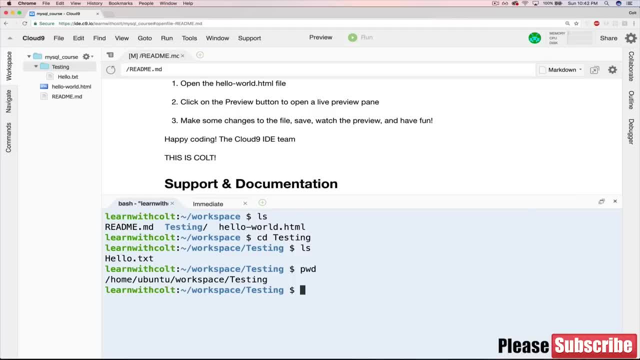 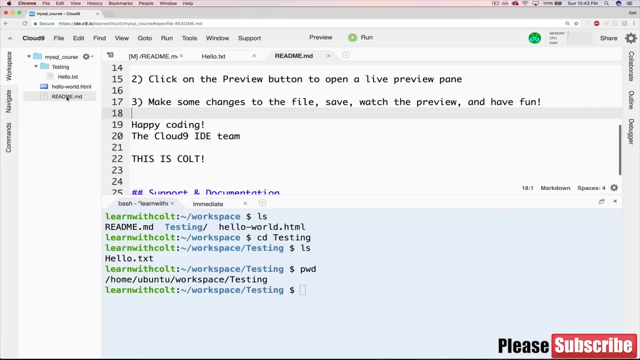 work with the MySQL interactive shell and a whole bunch of other things, But those will be MySQL specific commands, not the general bash commands. So that's pretty much all there is to the interface at this point. We have the file tree where we can double click to view files over in the editor. 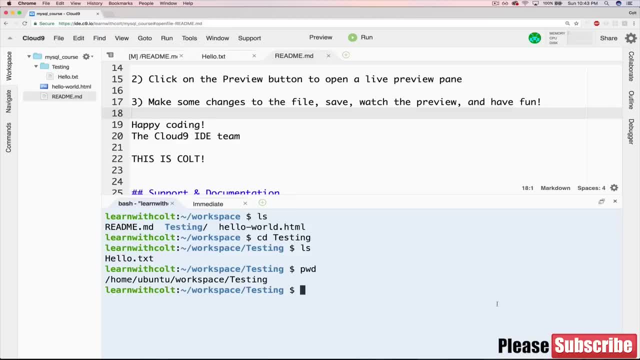 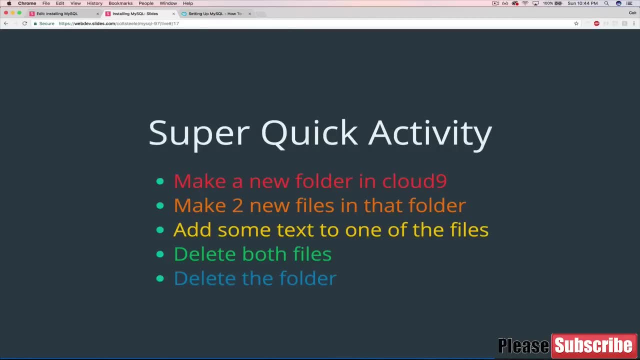 We can make changes there, And then we also have the terminal down here, which we'll be working with quite a bit as well. Next up, we have an optional, really really quick activity If you just want to get a little bit of practice with Cloud9, if you're feeling a little bit out of. 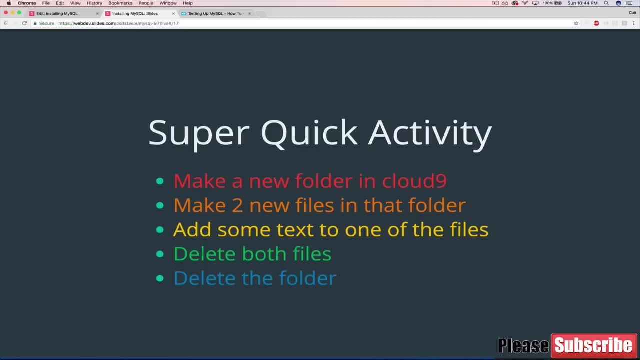 or uncomfortable with the interface. here's a really quick activity. So there's just five steps. Make a new folder in your Cloud9 workspace- call it whatever you want. Then, inside of that folder, create two new files, whatever type of file- txt is probably easiest- and name them. 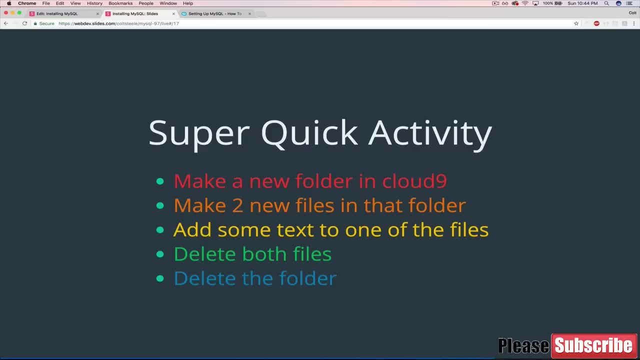 whatever you'd like. Add some text to one of the files and then delete both the files and then delete the folder. So not the most exciting, I know, But it's good practice. If you'd like to do that, go ahead and do it now, And then in just a couple. 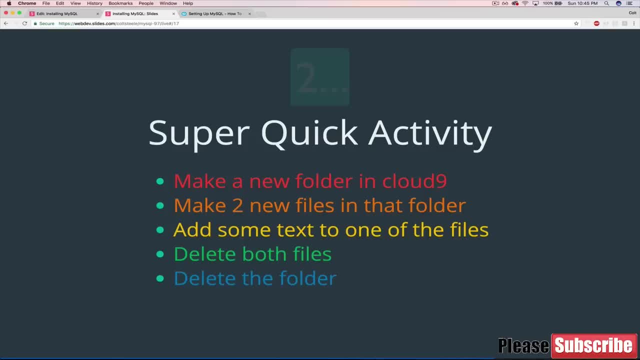 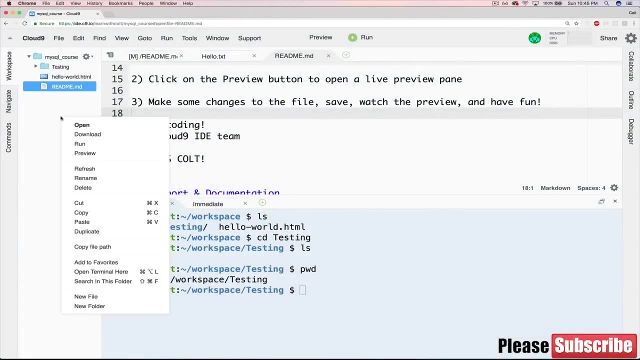 seconds, I'll have a solution. Three, two, one pencils down. All right, So to make a new folder, we can just right click new folder and we'll just call it my folder Then to make a new file. 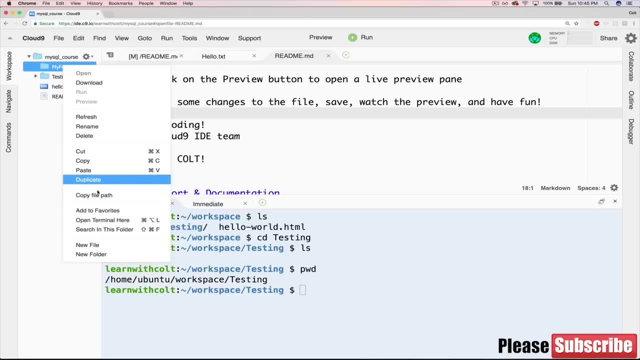 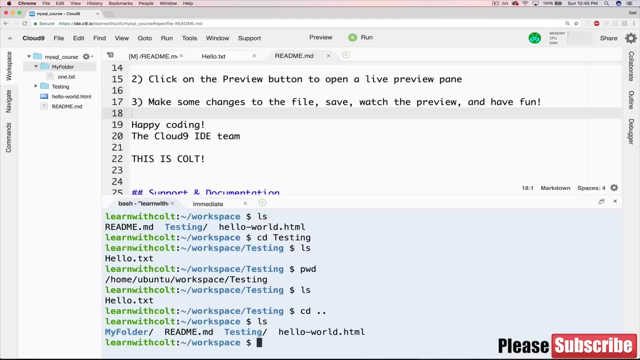 in that folder. we can right click again on the folder this time and we'll just call this one onetxt, and we'll create another one, And actually this time I'll show how to create it using the terminal, which is not a requirement. So I will navigate using cd and ls to my folder. 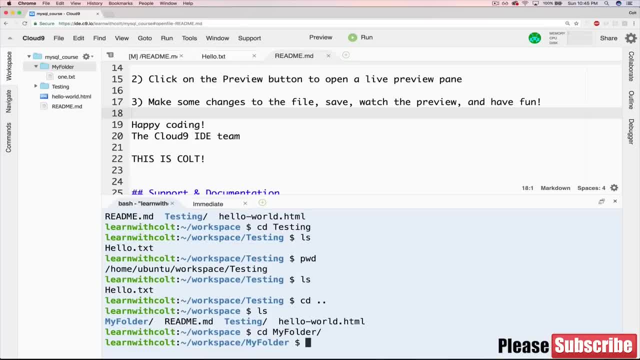 directory, Then inside of here I will create a new file called twotxt and I use the command touch. Again, don't freak out if you're not familiar with that. I'm just showing it to you just in case you are someone who likes to use the terminal. 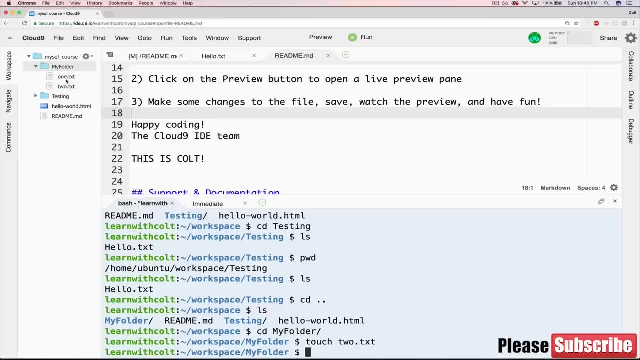 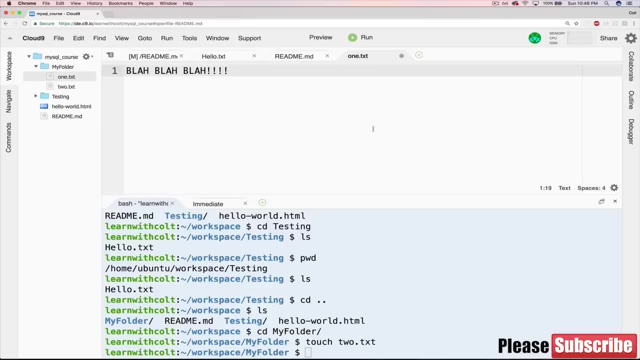 Okay, So that, as you can see, made a new file up here. Let's go into one of them, double click, add some text, blah, blah, blah. We'll save. close out of it, just to make sure it's there. Double click again. This other one's empty. Looks good, Now the next step is to delete. 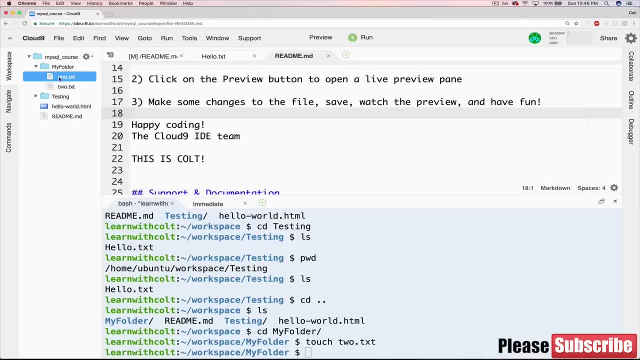 the files, And this is not something that I actually covered in the previous video, but I do think it's a pretty self-explanatory. You right click, you'll scroll down and click on delete. That's one way of doing it. It's going to ask you if you're sure you want to. 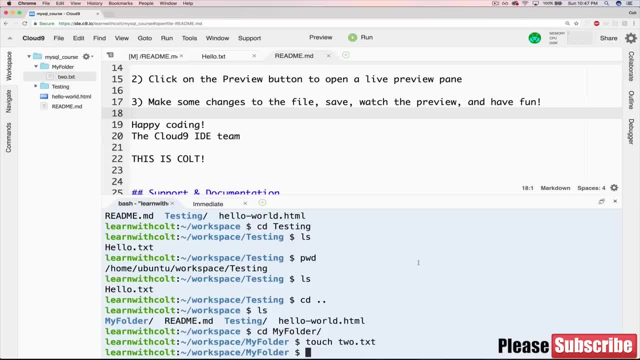 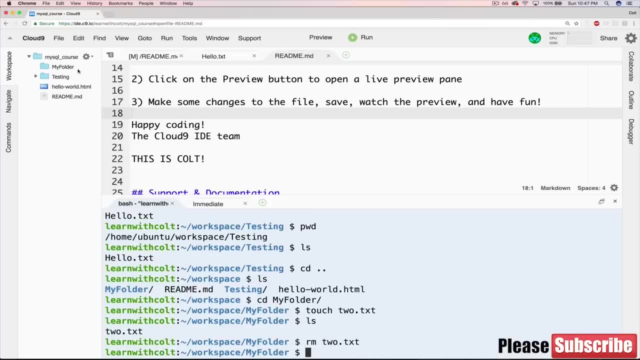 remove it. It can't be undone. We'll click yes, You can also use the command line. If that's something you'd like to do, use the rm command and you can see it disappeared. And then, lastly, delete the folder. right click and we can click on delete. You could. 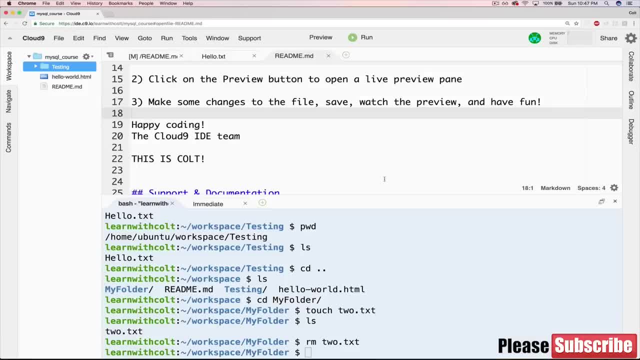 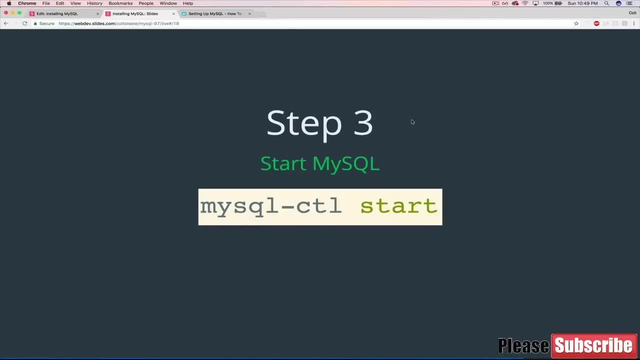 also do it from the command line as well, And that's it. So we finally arrived at the moment where we actually start working with MySQL, And by start working with, I mean we're just going to install it and make sure it's. 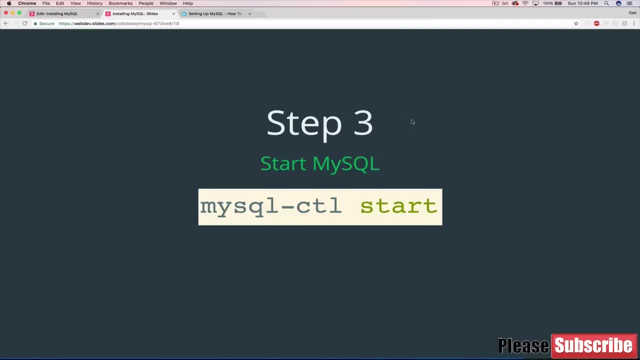 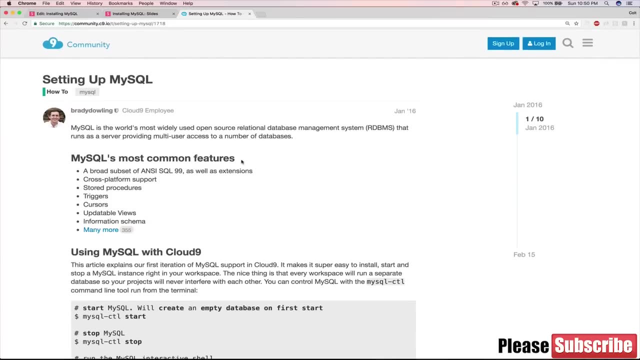 running correctly on our Cloud9 instance, But still it's something. So before we dive into that, I just want to show you a post on the Cloud9 community. This is written by one of the employees at Cloud9, and he's explaining how to use MySQL. 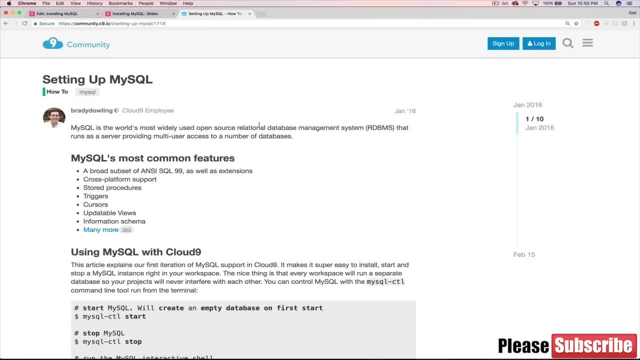 And basically what it talks about is that they've created at Cloud9 a really quick and easy way to get MySQL running in one of your workspaces. It's much, much easier than what you would need to do to install it on your own. They have a nice little shortcut There. 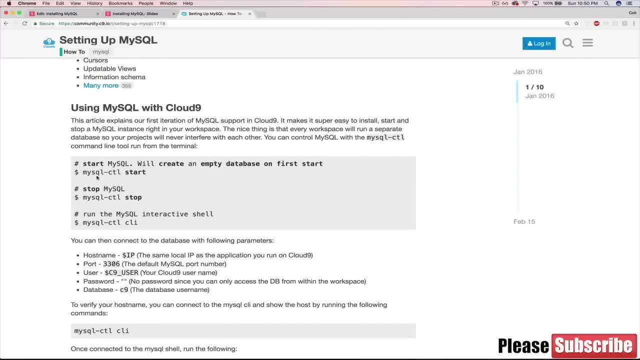 are three commands that we'll talk about. They're the three that are here Basically: start, stop and CLI. But before we go any further, let me just show you a couple of things that we can do. First of all, I just want to point out that these are not general MySQL commands that you 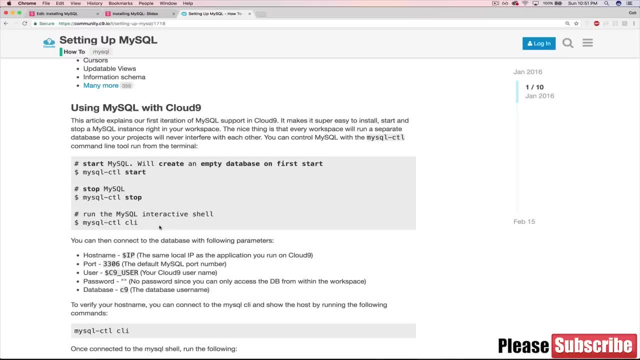 can run on any machine anywhere. These are actually Cloud9 specific, So the upside of this is that they've made it really really easy- like almost too easy- to get going with MySQL. You just run these commands and you're there. It's kind of magical. The slight downside of that: 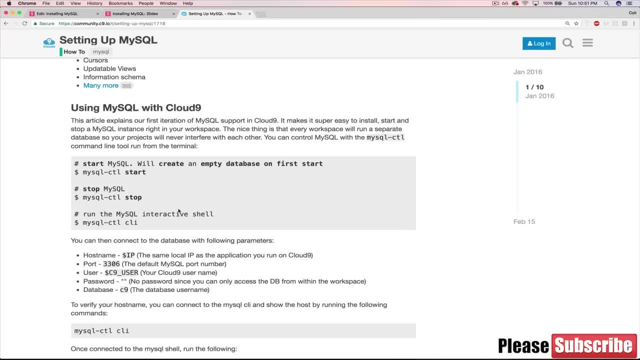 is that it doesn't work on every single machine and it is Cloud9 specific. So when you do install on a Mac or on a PC, you don't have to worry about it. You don't have to worry about it. You can just go through each one and see what works best for you. So you'll just have. 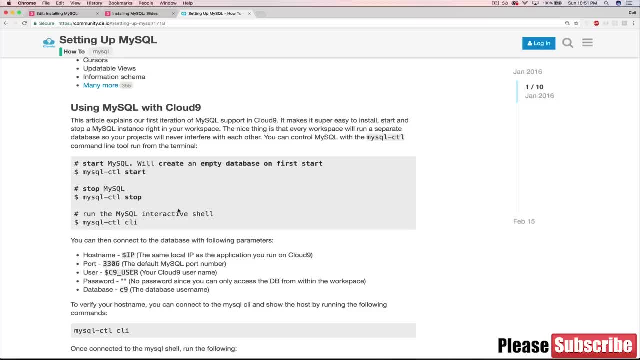 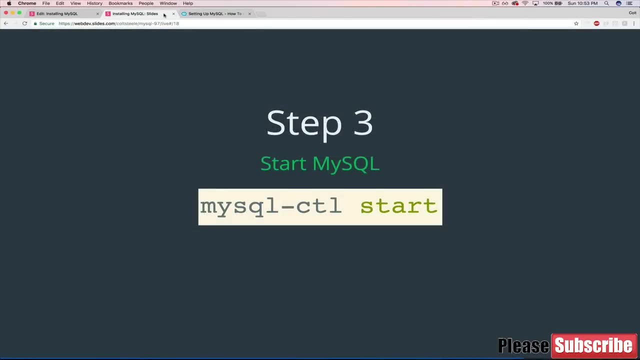 to relearn a new command to do basically the same thing, But for now, since we're in Cloud9, we get to appreciate how easy it is. So the first command is mysql-ctl- start And you'll notice that the three commands we're 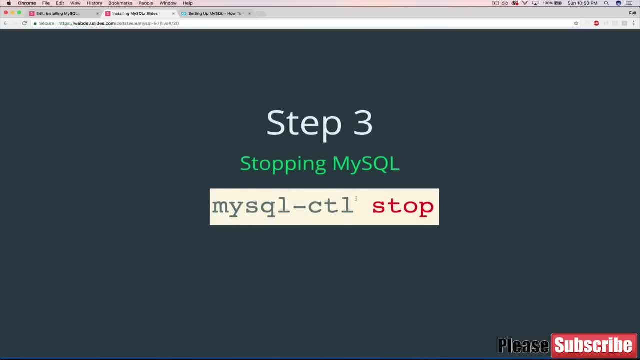 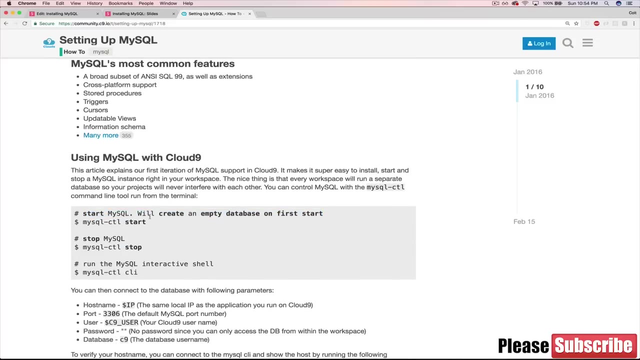 going to take a look at all. start with this mysql-ctl, And I believe it stands for command line tool ctl. It's just the abbreviation that Cloud9 came up with. So this first one. If we look at their documentation, it tells us it starts MySQL and it will create an. 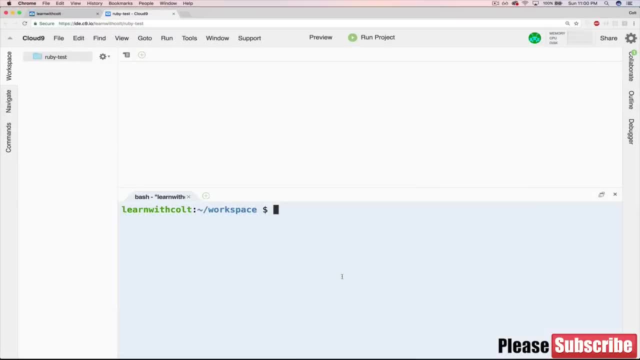 empty database the first time you start it, So let's give it a shot. You might notice that I cleared out everything in this directory. I got rid of those two starter files. You don't have to do that, but I just wanted to get rid of clutter. 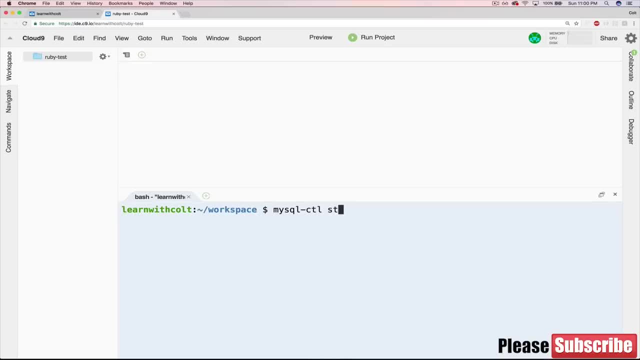 So we're going to write mysql-ctl start. You can see it's hard at work Starting MySQL. it's starting up a server. it's doing a few other things. don't need to worry too much about that. It tells us: a root user is my account name. database name is c9,. it created a database. 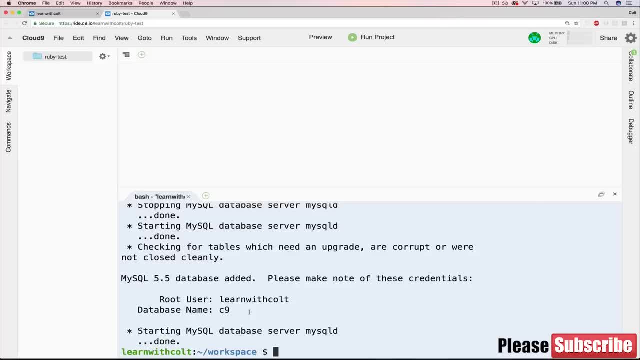 for us. Again. we'll dive more into this in the next section, when we actually start talking about databases and how you create them and work with tables and write SQL. For now, all that we really care about is that something happened, which is good. 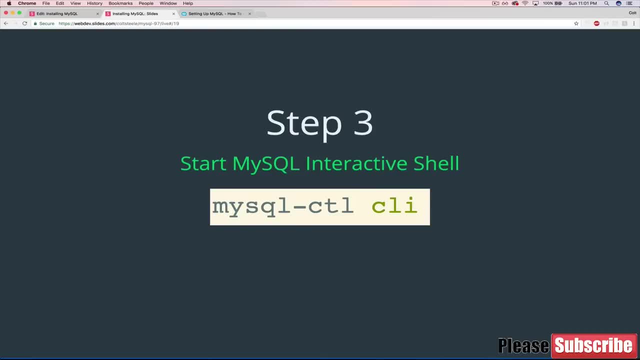 So the next command is the same thing: mysql-ctl- CLI, and that stands for Command Line Interface. What this will do is it will start up the MySQL interactive shell. If you've worked with any database before, usually there is an interactive shell that 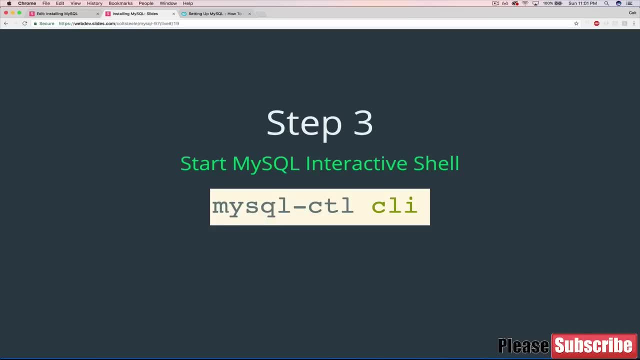 goes along with it, Or if you've worked with things like Ruby or Python or Node. there are usually terminal or command line based interactive environments. If this is all new to you, go ahead and try it out. Thanks for watching. I'll see you next time. 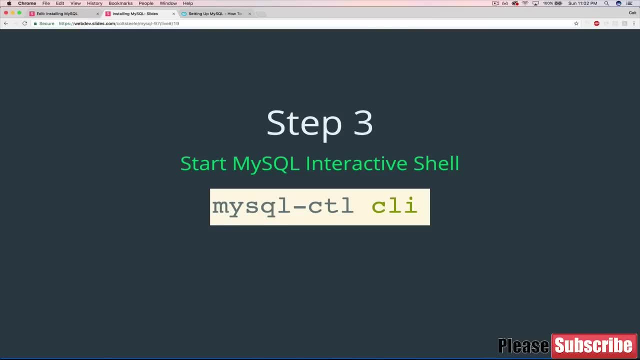 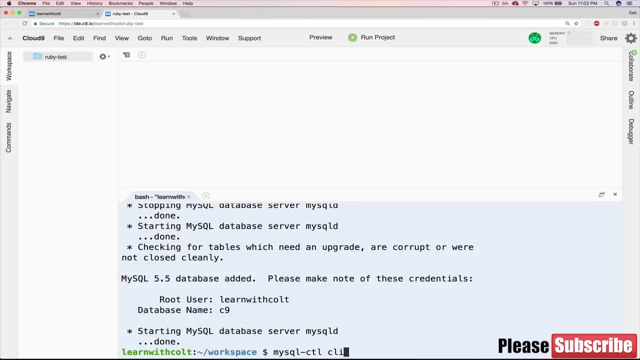 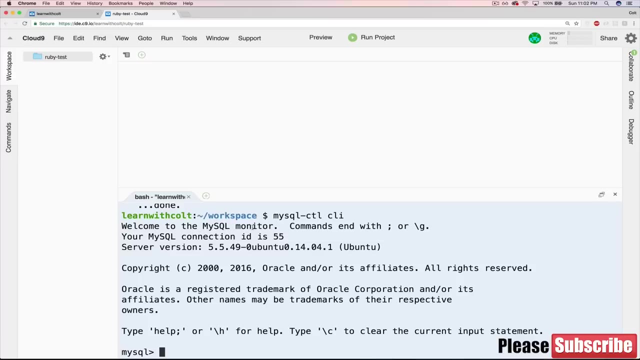 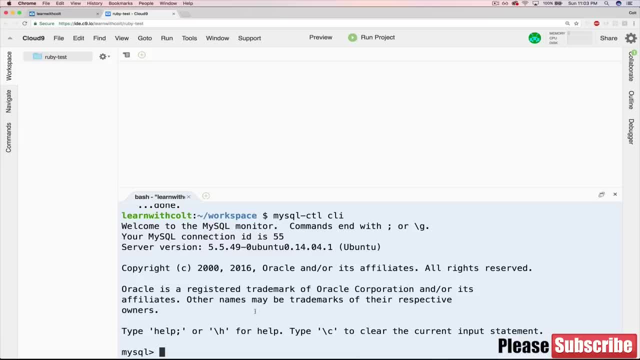 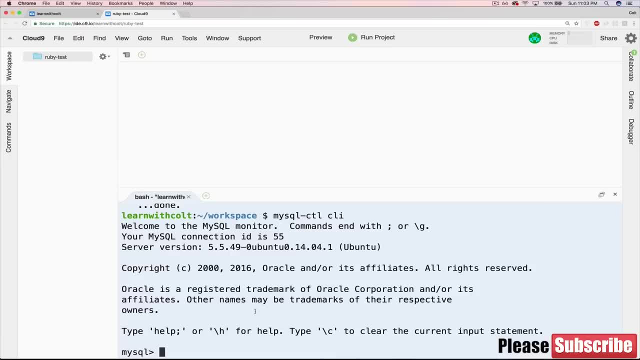 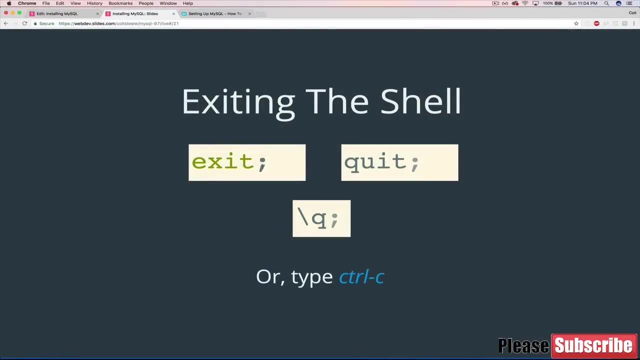 Bye, Bye, Bye, Bye, Bye, Bye, Bye. All that we're going to see right now is that you can quit this. There are quite a few ways of quitting the shell. We can use exit. notice a semicolon. quit also. notice a semicolon. 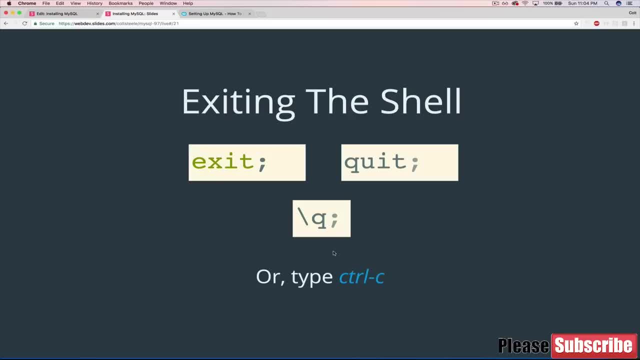 We can use backslash Q. I always mix up forward and backslash, but this slash pointing down Q or what I usually use, control C. So whatever works best for you, I think there are actually a couple more different ways. 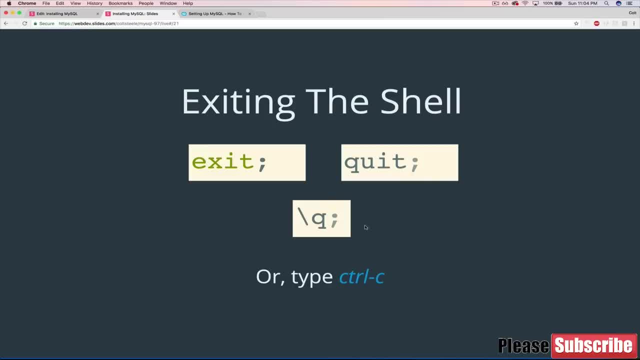 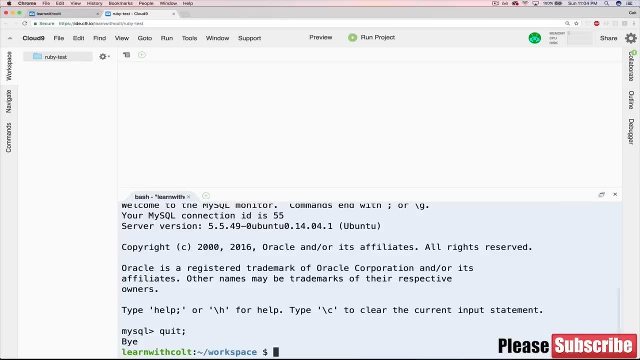 of quitting, depending on the platform you're using, But for me I usually use control C. But just to illustrate that I'll do two of them. So let's do quit semicolon. we get a nice message. bye, seems a little sad. 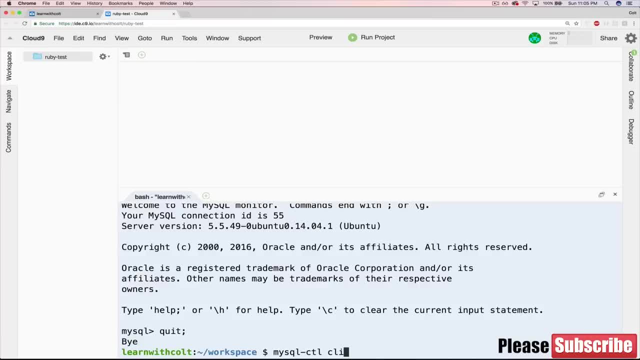 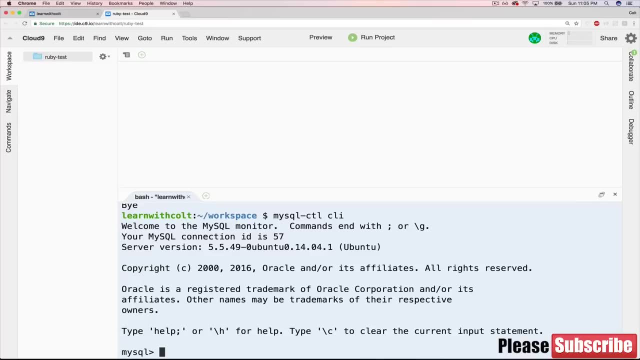 We can restart the CLI by either retyping that whole thing or just hitting the up arrow. So I'm going to do that now and hit enter. We get this. exactly. It's the exact same message. You'll see it every time. 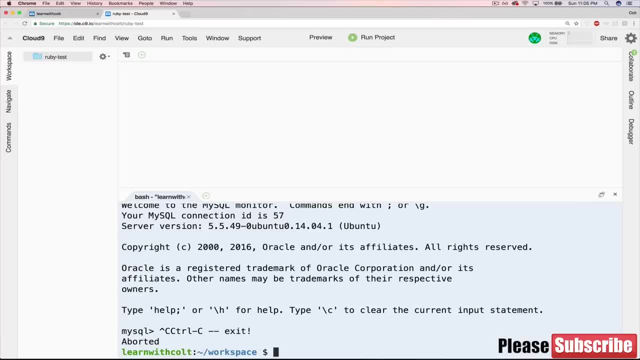 This time I'm going to use control C. You'll just have to trust me. I did it. Actually you won't, because you can see it here: Control C. this time it says aborted. So it turns out there actually is a little bit of a difference. 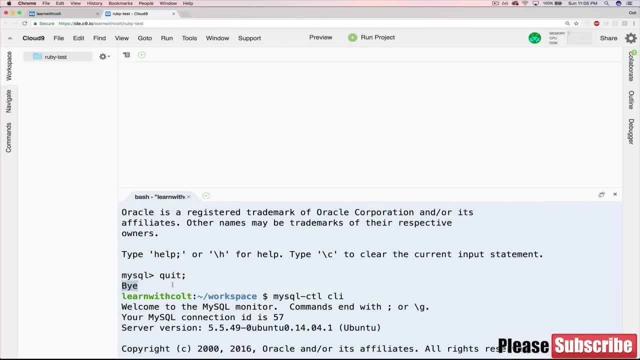 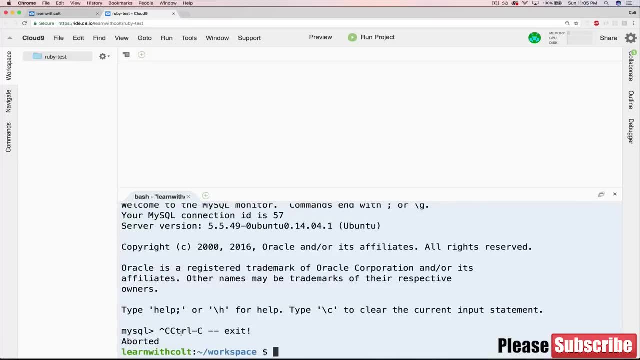 If you notice up here, it said bye. It kind of was expecting to quit because I used the quit command And here I just ended the process, which is why it says aborted. So technically there's a difference. But I just used control C because you don't have to really type anything. 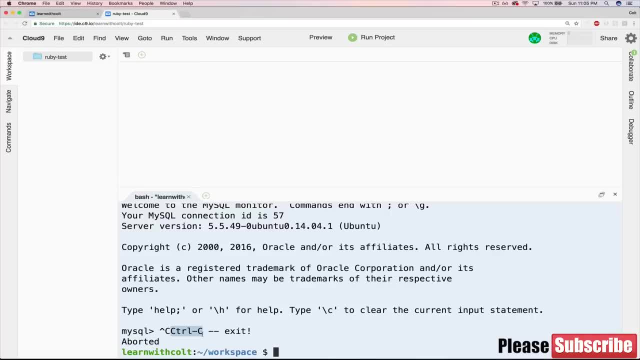 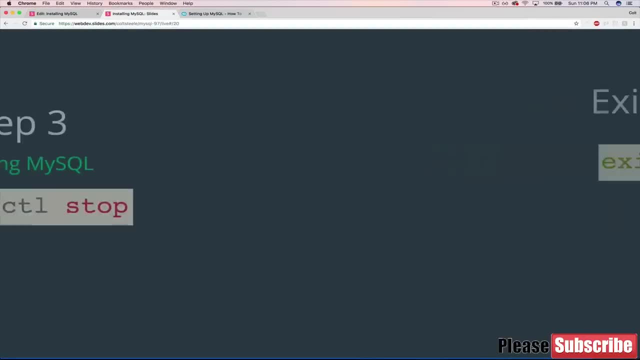 It's much easier. You don't have to hit the enter key, You don't need a semicolon. Really, whatever you prefer. Some people like to be more explicit and use quit or exit. Okay, So the last command that we're going to take a look at is mysql-ctl- stop. 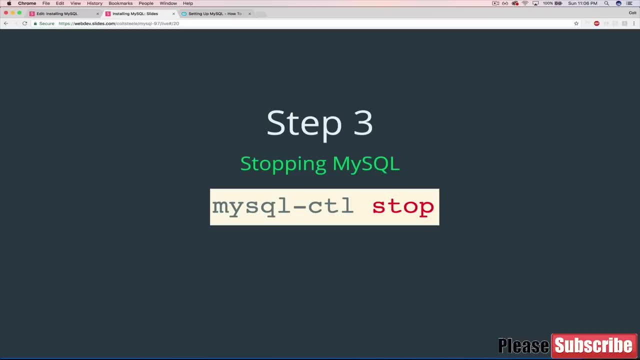 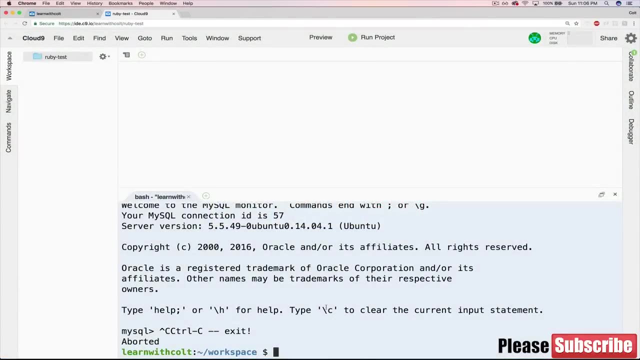 And you're really, really rarely going to use this one. But what this one will do is stop the mysql process Completely. So to understand what that means, it helps to understand what happened when we typed this first command here. that started everything. 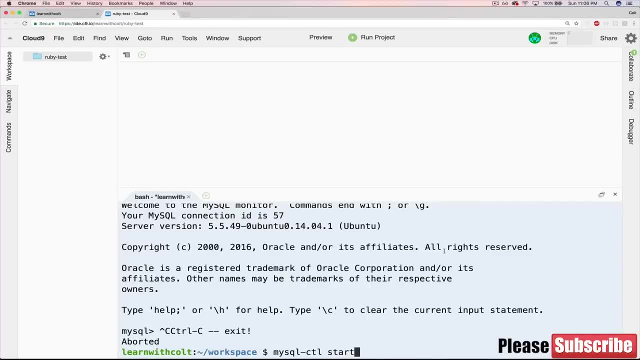 So what that did is that it started up a new instance of mysql. Then that's running constantly in the background at all times until we stop it When we use this second command, mysql-ctl-cli. I know it's a lot of abbreviations here. 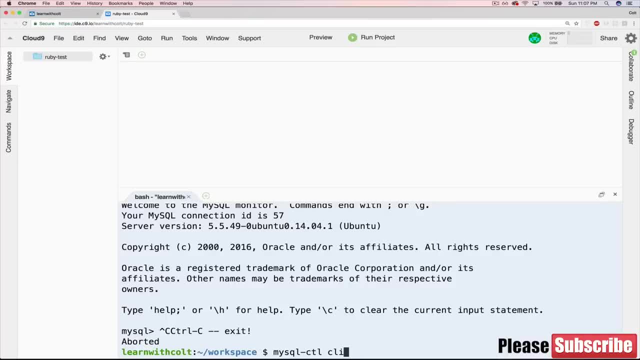 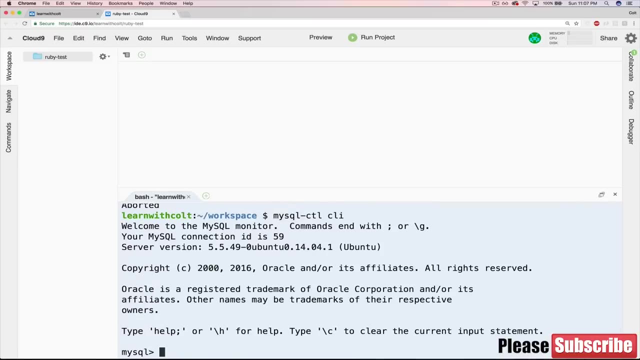 But when we use that cli command it is connecting to the instance of mysql that was started up from the first command. So just to reiterate this cli, when we do this and start it up, it is connecting to mysql connection that we started up earlier. 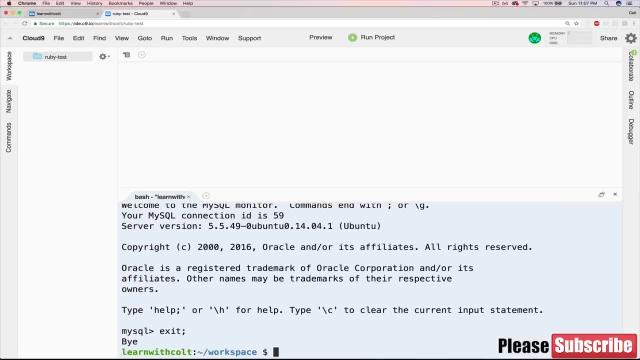 So I'll exit And, if we wanted to, we can stop that background process. We can stop mysql from running completely. So we're not just stopping the cli- This is already stopped here- But we can stop everything related to mysql using mysql-ctl stop. 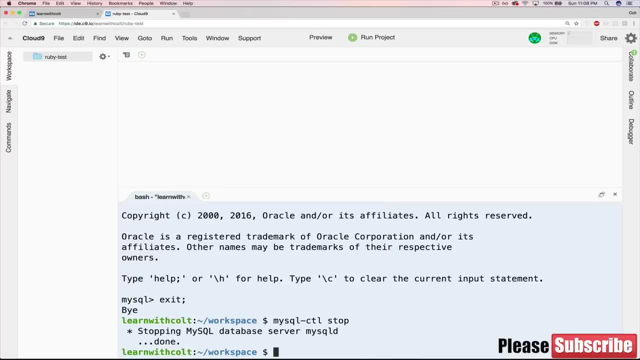 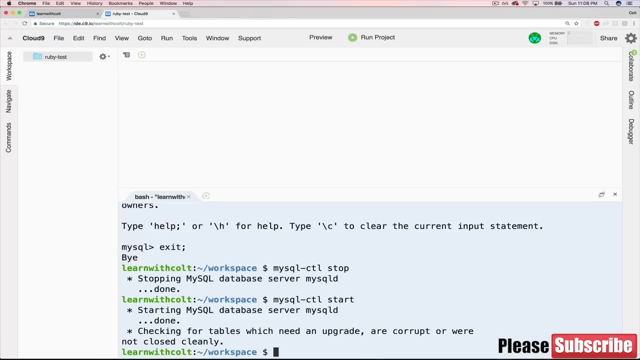 And it just tells us stopping mysql database server. blah, blah, blah. Okay, so three commands. Realistically, the way that this will work is that we'll start it up and we're going to leave it running for basically the entire course. 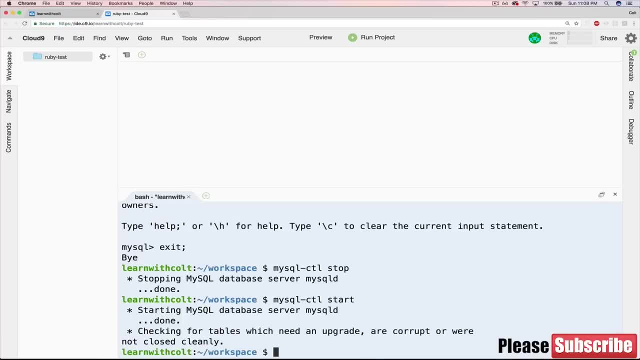 And we're going to start and stop the cli all the time. Pretty much every other video will be starting up the cli typing some code, quitting, So you should get used to that, But you don't really need to worry about stopping it all that often. 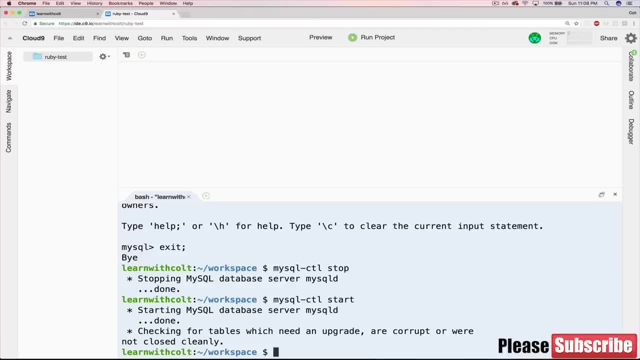 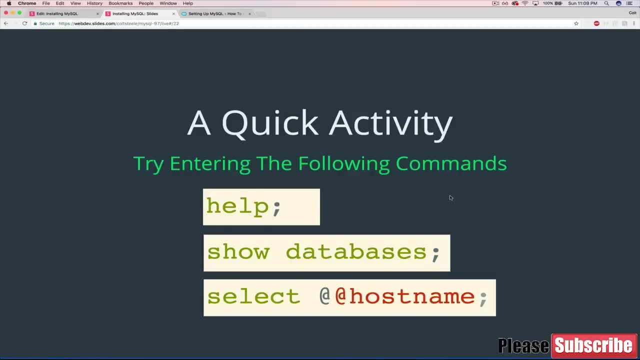 Okay. so next up, we just have a quick little exploratory activity where you'll be able to type some new commands into the cli and see what happens. Okay, so, as I mentioned in the last video, we're going to do a really quick activity where you're basically going to try. 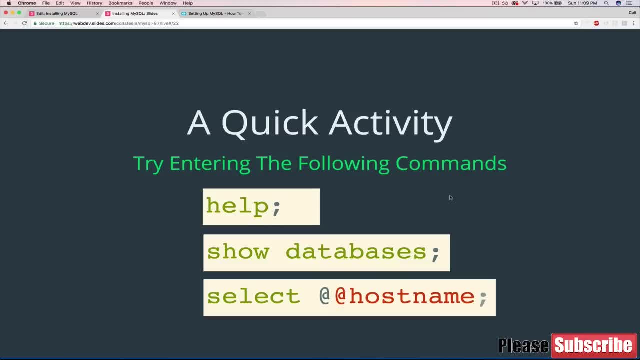 experimenting with these three commands and enter them into the mysql-cli. So if you stopped it, if you quit, make sure that you open it back up using the cli command And then try running these one at a time and just see what happens. 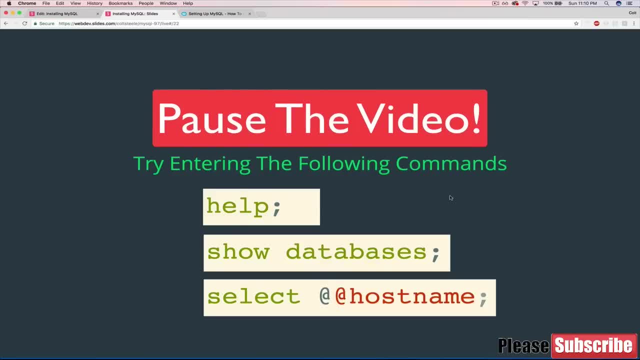 So pause the video, if you'd like, and do that, And then come back and in a few seconds we'll go over what happens. All right, so let's start with the first one. help. So I'm going to clean up my cli. 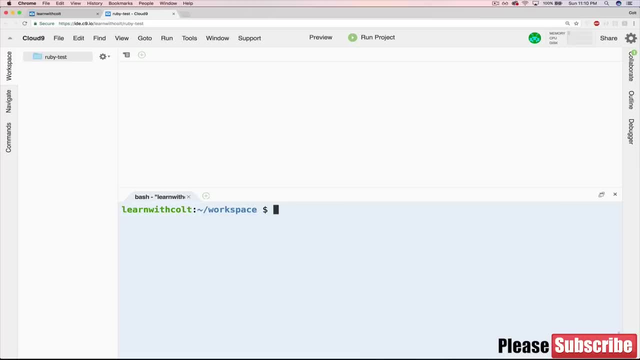 I'm going to clean up my terminal here just by using the clear command. Then I'm going to access the cli. I'll just use the up arrow. So now I have this cli command line interface ready for me to type some commands. So I will do that first one, which is help. 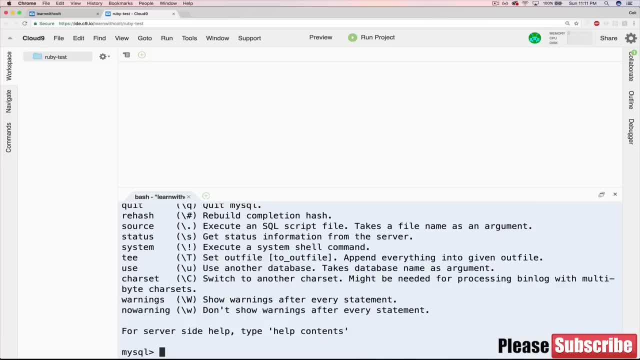 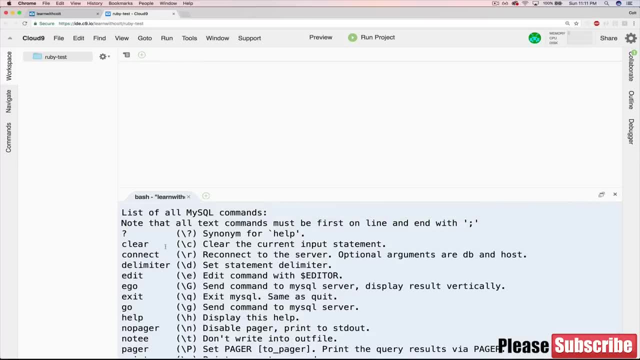 And you can see we're actually prompted to type that. So when I hit enter, all it does is give me a list of commands that I can do. You can see we've got things like clear help, which we just used: print prompt. 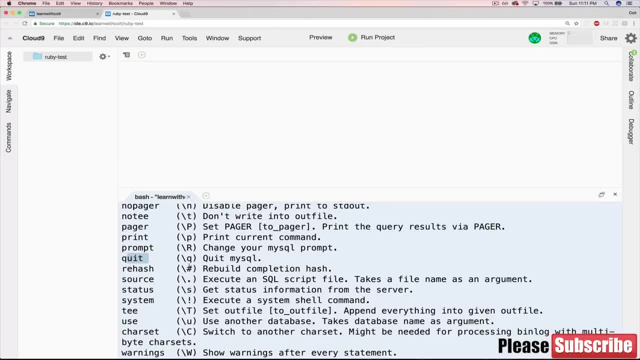 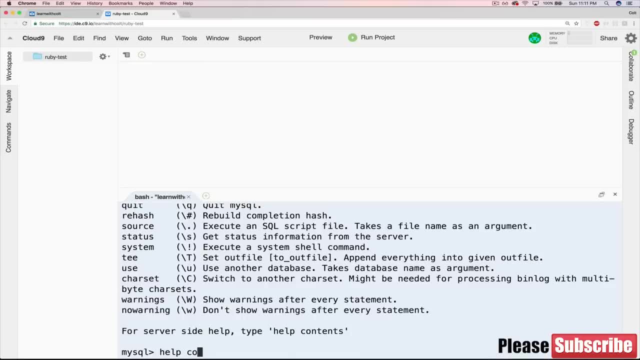 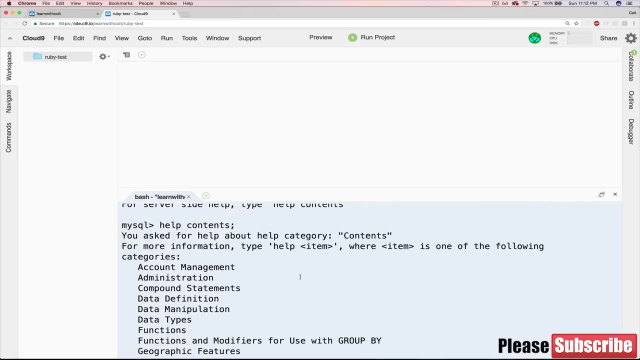 We've got quit, which we already used as well. Basically, it's just a list of things that you can do. As you can see, we can also try help contents And we basically get a list of categories that we could access. 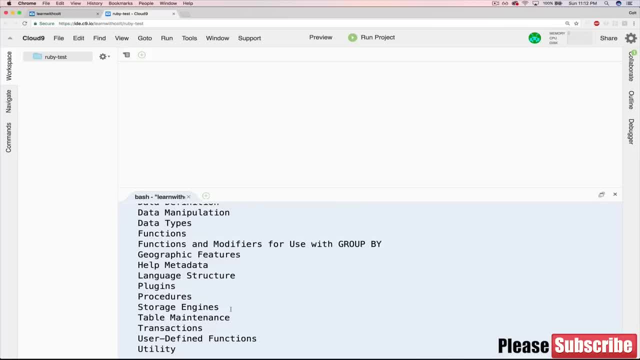 So if we wanted to know more about, let's say, let's just pick one of these at random, Don't worry, Let's try data types. We can do help data types And it kind of dives down further and gives us information about what those are. 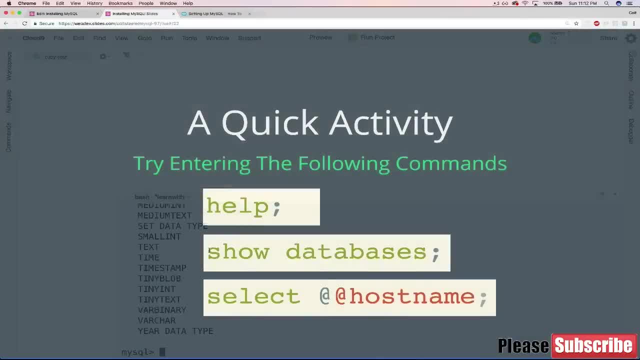 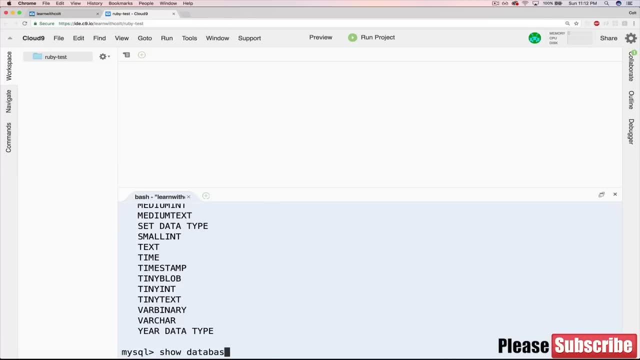 We haven't talked about data types, so don't stress about that. The next command to try is show databases, So we'll come back. try that show databases And it gives us this nice little representation Here of the current databases that we have in this instance of MySQL. 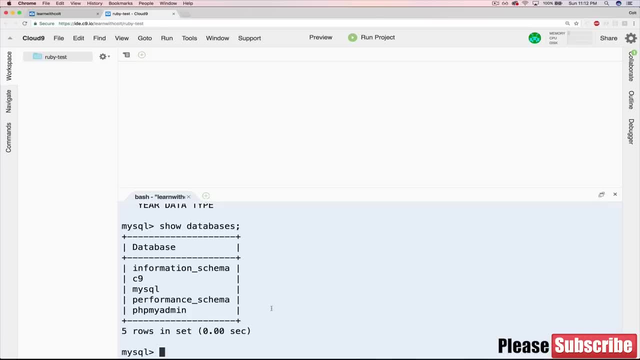 So we haven't talked about how you make a new database. You might be wondering what's going on. There's already five of them here. All of those were created automatically when we created this MySQL instance, So, don't worry, It doesn't really matter what they are right now. 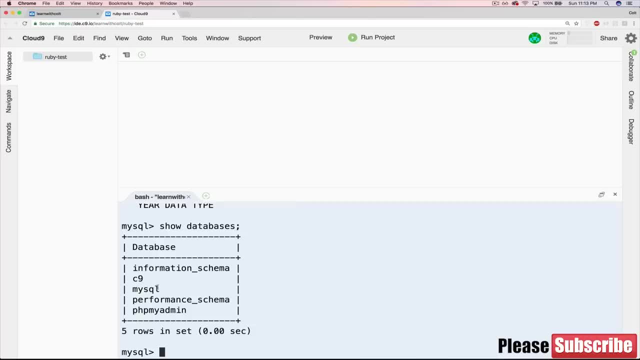 But they're there automatically. There are five different databases. In the next section we'll actually talk about what a database is, when you create a new database and how it works, Why you create a new one when you use the same one. 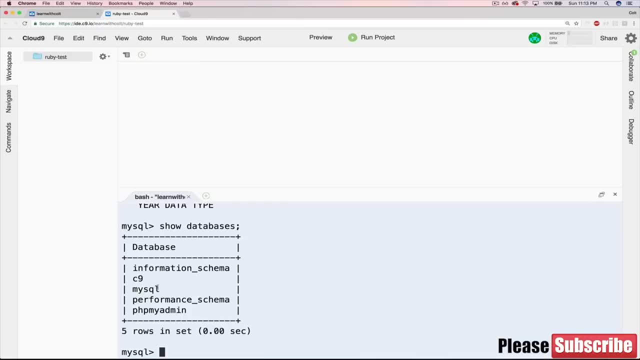 But I just wanted to show you this command because you'll be able to use it in the future When you create a new database and you want to make sure it worked. you can type show databases and you should see a new one added below. 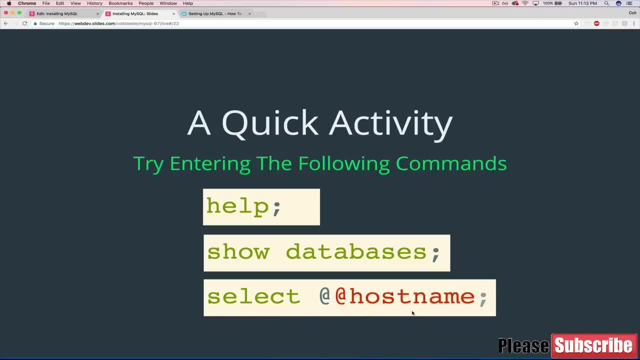 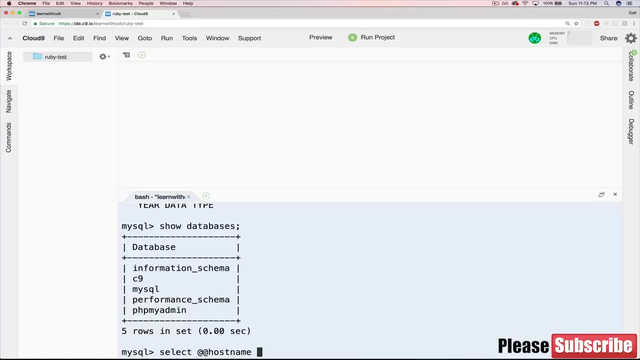 And the final command here is select at at hostname. This is also kind of a weird one that most likely you will never type after this, But I just wanted to show it to you, Not because it's something you need to do, But just it's something that you can do quickly and immediately. 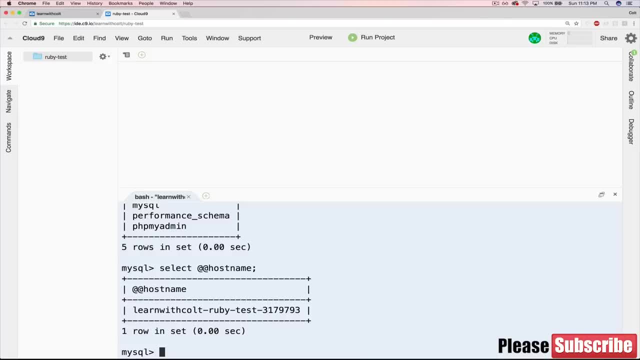 And all of this here is just to illustrate the point that the CLI works by you typing commands, hitting enter and getting some text back, So that process over and over and over. So here it tells me that my at hostname is this string here: 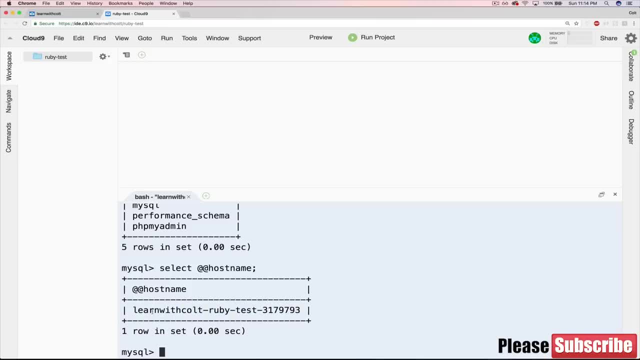 Basically my username. Yours will be different depending on your workspace and your username. So, as I mentioned, it's honestly not important what it is Okay Or why it's there at this point, But I just wanted you to see that you can type these commands in and get something back out. 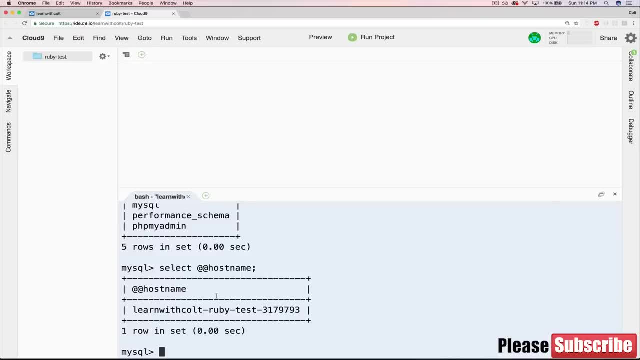 So that's it for this really quick kind of silly exercise, But in the next section we're going to start actually learning SQL commands So you'll be able to start interacting immediately: Creating databases, creating new tables, adding data into those tables. 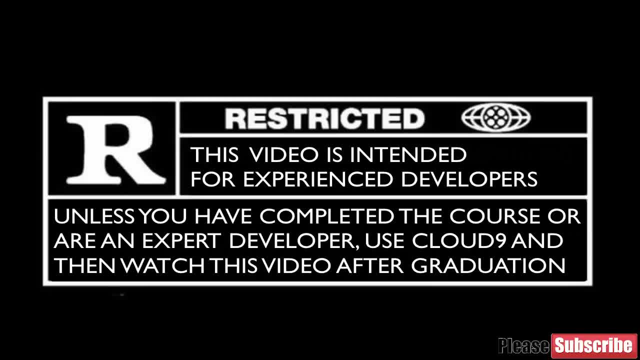 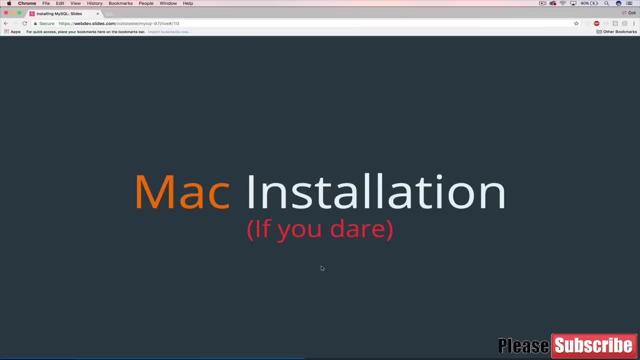 And it gets a lot more interesting than I promised. Warning: This video may contain extremely frustrating installation instructions And it's for experienced developers only. It's advised that you install using Cloud9 to avoid needless pain and anger. Okay, Welcome to this video on installing MySQL on a Mac. 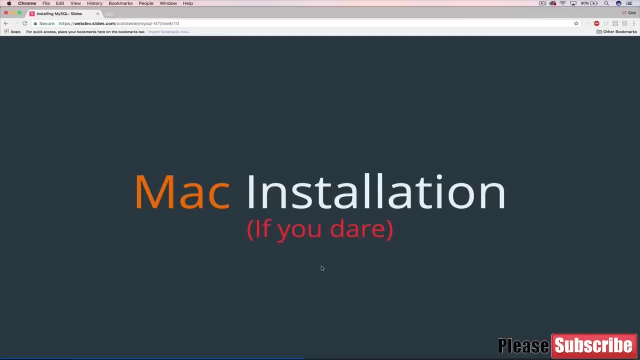 And again, I'll warn you, this can be painful, And this lecture and doing this, all these steps are 100% optional. In fact, if you don't have a good reason, if you're not sure if you should do this, then that means that you shouldn't do it. 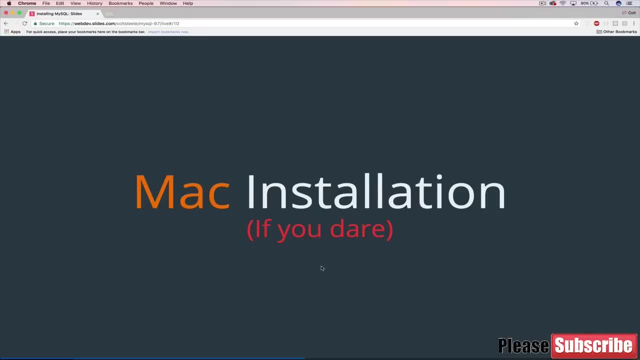 At least not until you get to the end of the course. Of course. if you're somebody who is an experienced developer and you know you want to get this running locally at the beginning on your Mac, then go ahead, follow these instructions. 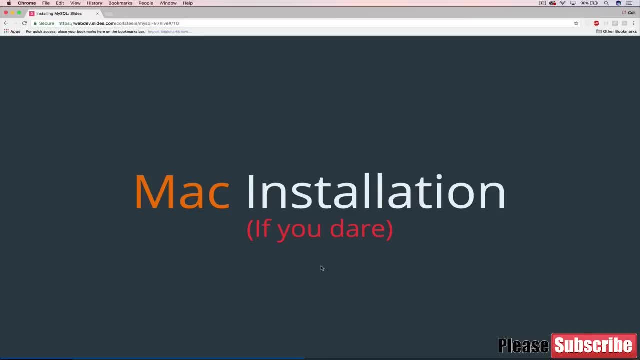 But I would definitely recommend that you go through the course, for 99.9% of the people in this class. Go through the course of Cloud9. And then install this on your Mac at the end. It just makes everything so much easier. 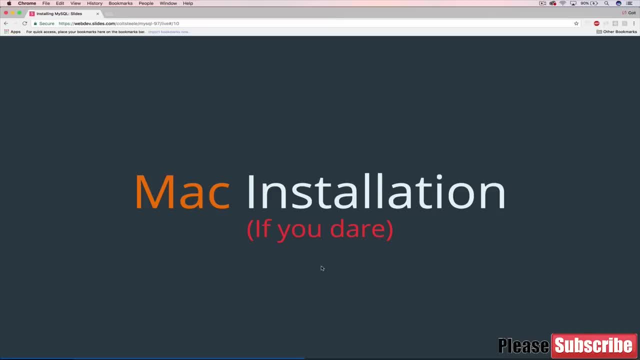 Okay. So if you're still here, though, the steps to actually install it are surprisingly simple. The problem is, once you install it, you run into issues, Depending on your developer environment, Depending on things like if you're using Bash or ZShell. 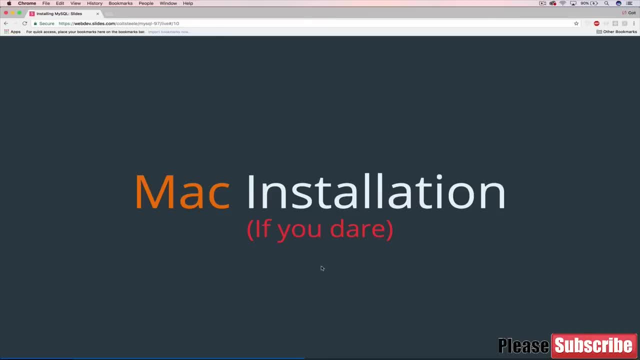 If you have permissions issues and passwords, It just turns into a nightmare a little bit- Well, not just a little bit, a lot. So the first thing we need to do, like I said, is actually nice and easy: Just go to mysqlcom. 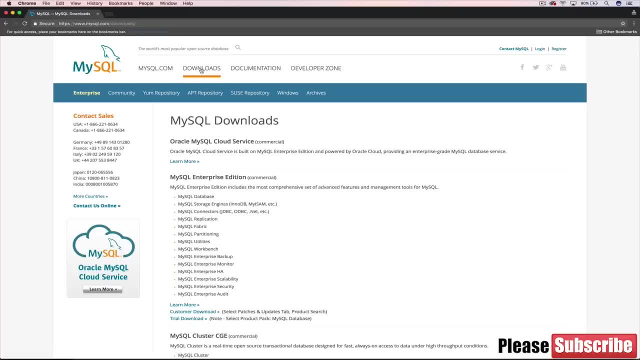 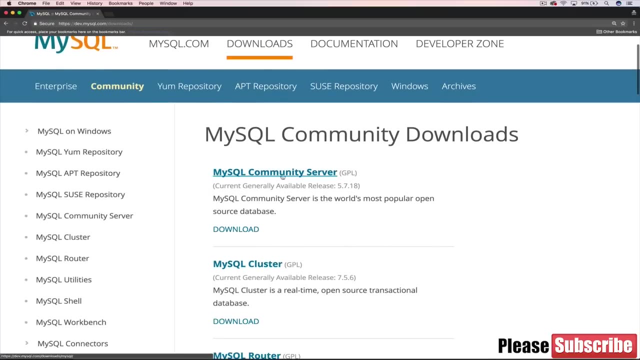 Go to the Downloads tab And what you'll see here are a bunch of the basically like the commercial services And MySQL Enterprise software that is not free. We want the Community section And then we want the first thing here: MySQL Community Server. 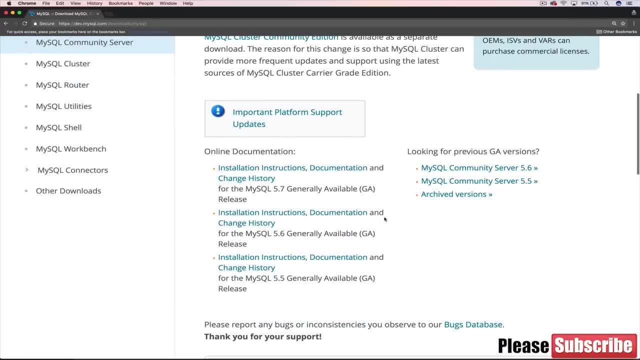 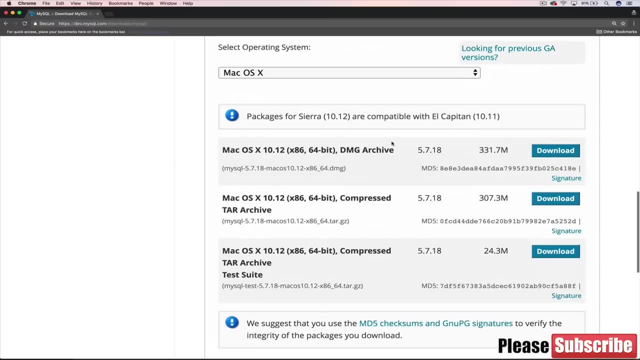 Then at the very beginning- this is kind of just a blurb about it- Some documentation instructions, But if you keep scrolling down you'll see the download links. So you'll need to select the one that corresponds to your Mac, Depending on how old your Mac is, how new it is. 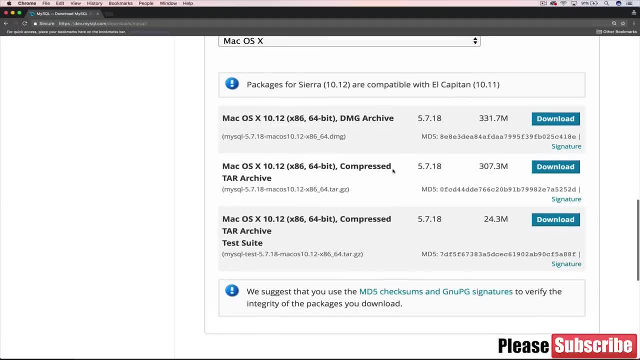 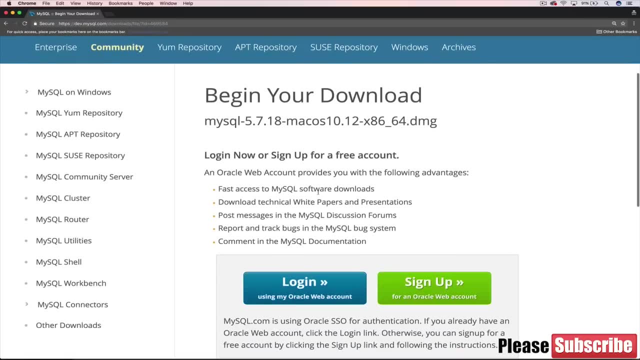 What version of Mac OS it's running. All of that, You'll have to make a decision, But for me it's this first one here, So I'll click Download And it looks like you have to type or you have to sign in or create an account. 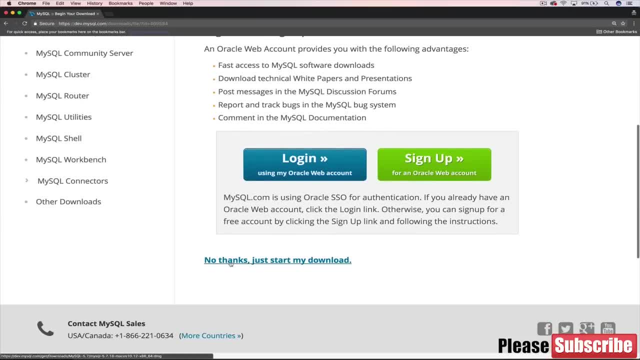 But that's not true. You scroll down and there's this link: No thanks, just start my download. Of course, if you want to, you can sign up, But most of you probably don't care, So just click No thanks, just start my download. 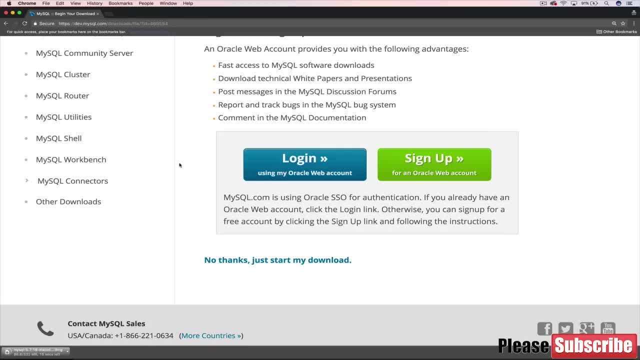 And I'll see you in just a second, Once I edit this download timeout. All right, Now that's completed downloading, So I'm just going to open it up. It might take a second to open, But once it does, you'll see a single file inside of this. 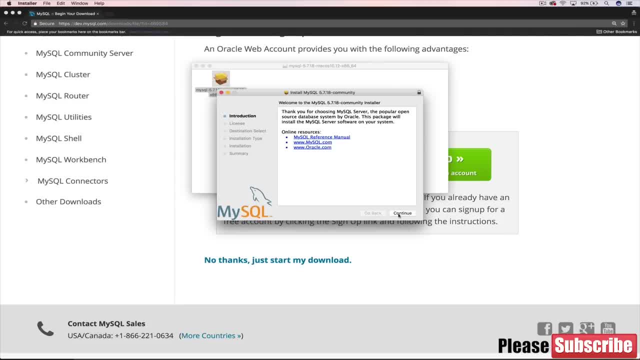 And we'll just double click, Follow the steps, Continue, Read every word of this. Of course, I've already done it, So you know. I know everything it says. Click Agree Tells you 1.13 gigs of space needed. 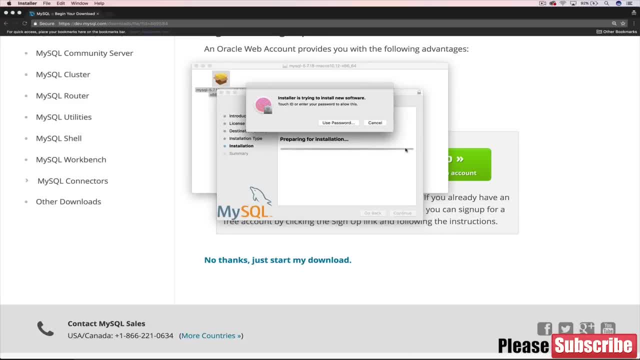 So make sure you do that, Make sure that you have that available. Then we'll click Install. Then it will ask you for your password for your computer. Fortunately, I guess I can use my thumb or my finger, That way you don't have to watch me type my password. 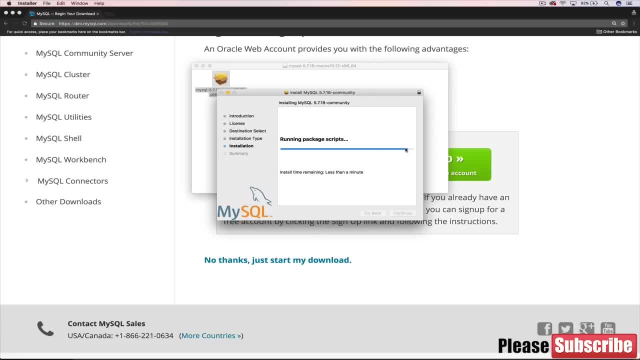 I don't have to edit that out, It's always a problem. I don't want people to see my passwords, Okay, So here's an important part. I mean it's all important, But this in particular. it gives you a little pop-up here that says: 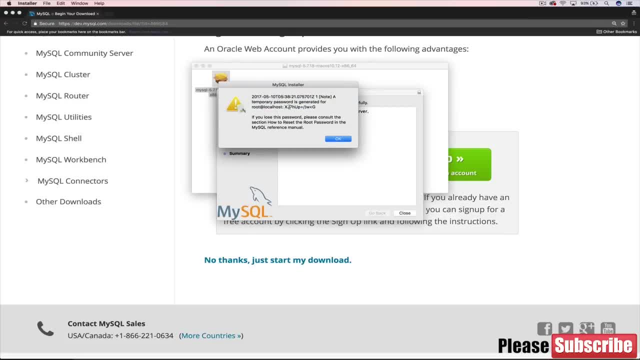 A temporary password is generated for root at localhost And then it gives you this password. So I highly well, I don't highly recommend it. You need to copy this Technically. if you forget it or you lose it, you can reset the root password. 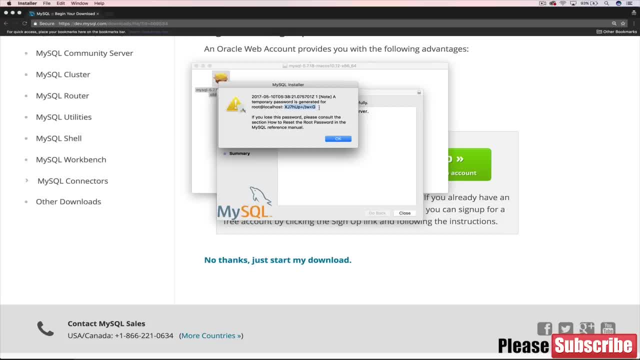 It's just another set of steps and complications. So copy this, Save it. Okay, We're now done installing it. I'm going to move it to the trash. So we're done with the install. But that's the easy part. 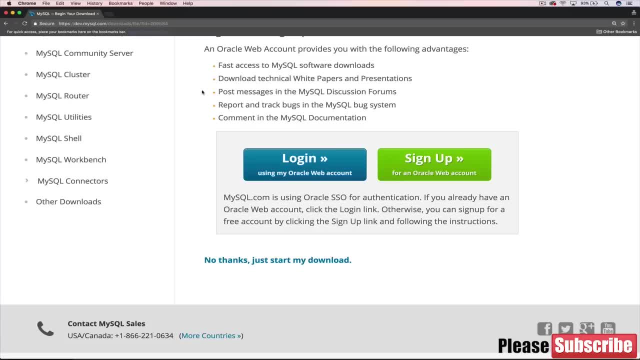 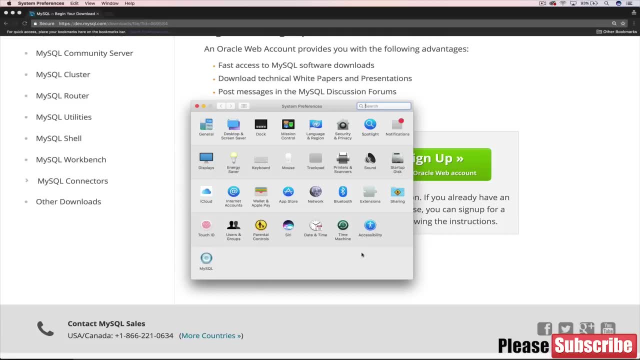 Just do it, Just a couple of clicks. Now we need to do a couple of things. The first is start up the server. So to do that we go to System Preferences And it should be down here. There should be a new icon somewhere at least, depending on how you have your setup. 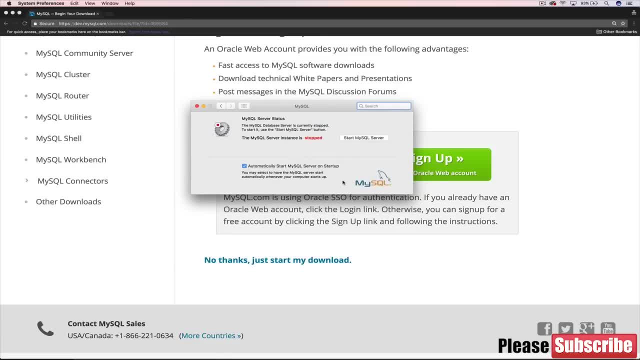 For me it's the bottom left, MySQL. I'll click on that And we should see MySQL server status. you know, blah, blah, blah. The server instance is currently stopped. There's a button to click to start it, which will start it. 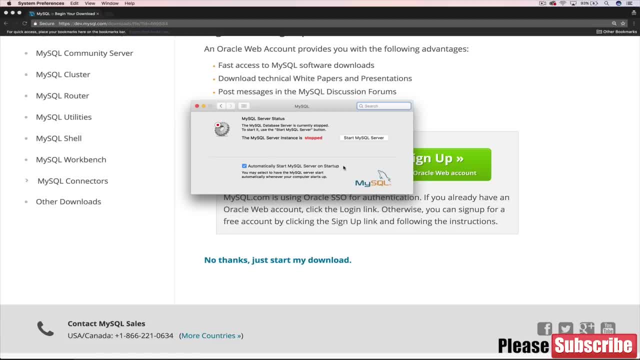 And then there's also this checkbox which I'll address now. Depending on what you want, you can have MySQL server start up every time you start your computer. I'm not going to do that. You have to type your password again. I have like six or seven database servers on here. 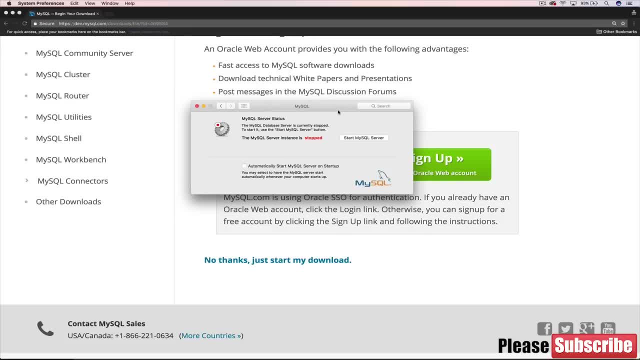 And I just don't want any of them to start up on this machine. at least, This is not my developer machine. This is what I use for teaching. Totally up to you. It just depends on how you're using it. But if you're just learning MySQL now, 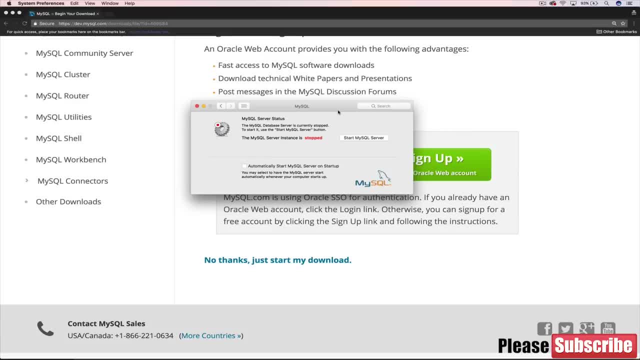 it might actually be good to leave that on so you don't have to continually start it, But either way, it's not that hard to start. It's just a button here which we'll click now And there we go. If you didn't click this or uncheck this, 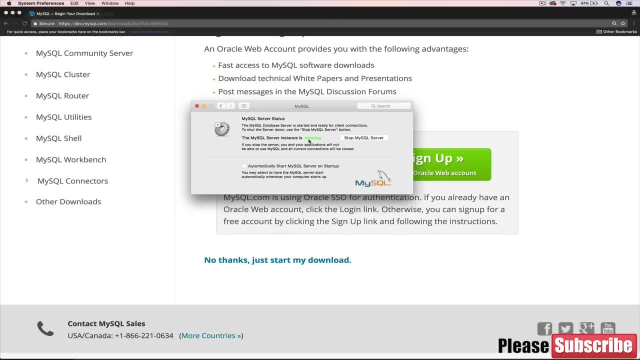 you may have to type your password when you click that the first time. Okay, So now what we have left to do is open up our terminal and start interacting with this. So I'm going to bring the font size up a bit And, theoretically, 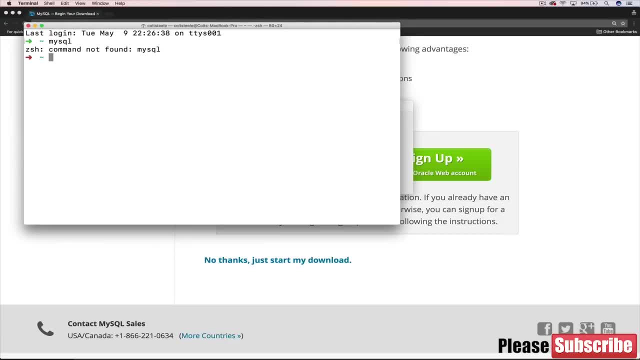 you should be able to type MySQL, But this is where we start running into issues, So I'm getting this command not found And if you get this again, this depends on how your Mac is set up and your developer environment, And this is where it's annoying. 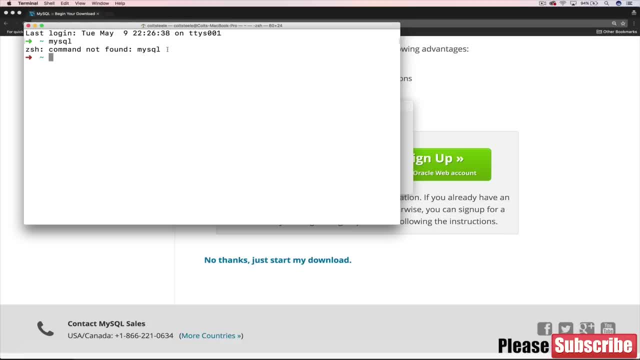 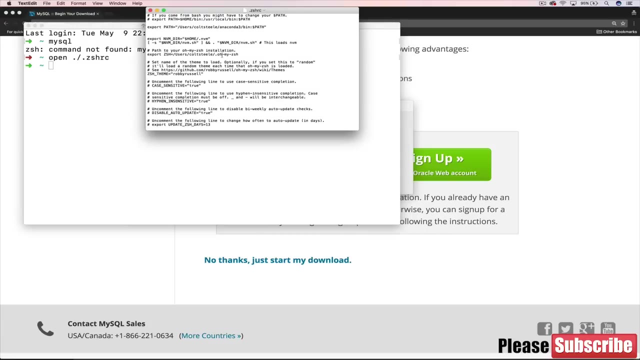 But for me I'm using something called ZShell. I'm getting command not found, And that's because the MySQL command is not in my path. So what I need to do now I'll open up my slash dot zh rc file. 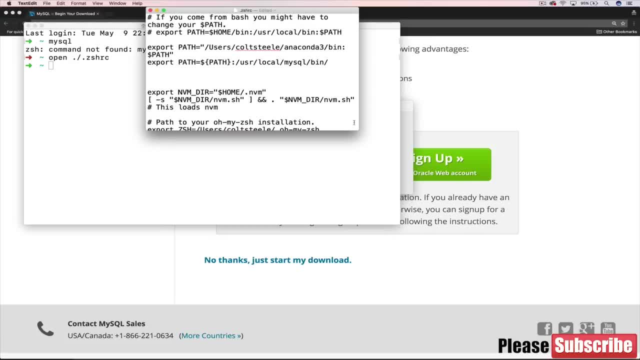 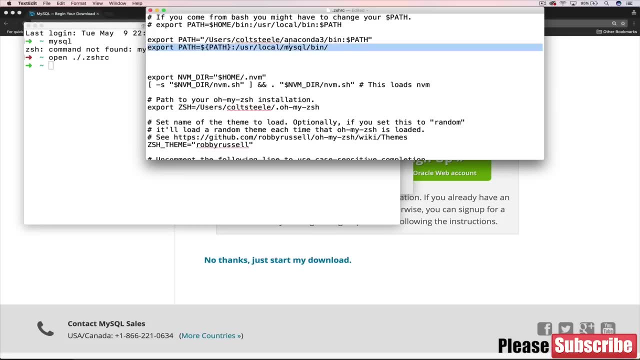 And I'll paste this line in here just so you can see it. I'll include this in the instructions for this lecture. You can find this on anywhere online. It's a very common error when people type MySQL and you get command not found. 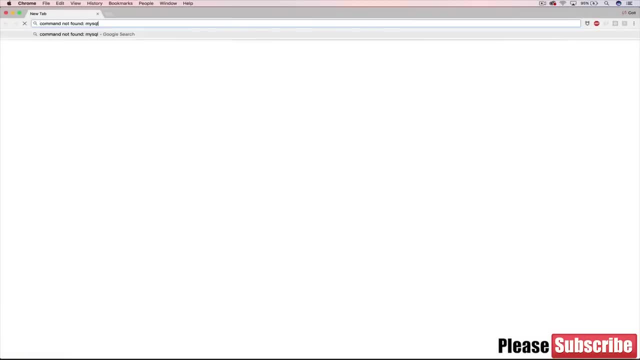 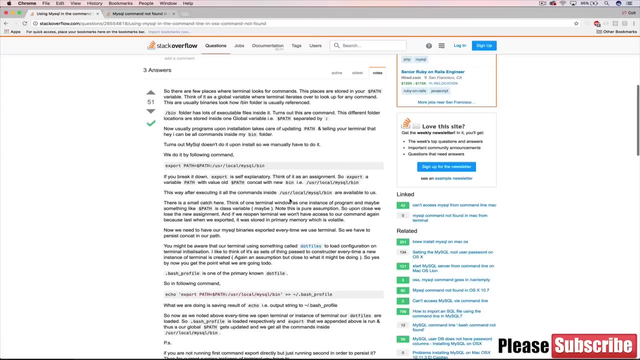 In fact, if we just did that right now and went to Google, you can see, depending on you know what version of osx you're running. there's all sorts of replies that are basically exactly what i just did. in fact, that's where i got the line originally. it just depends. 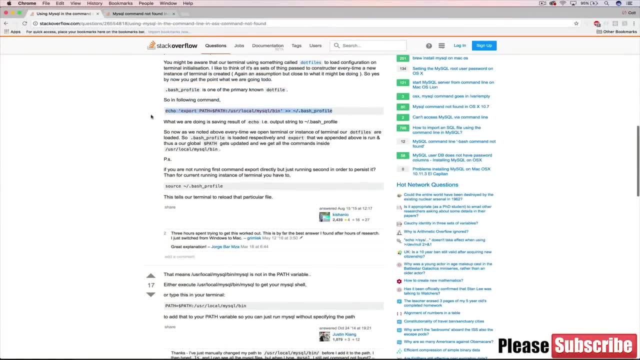 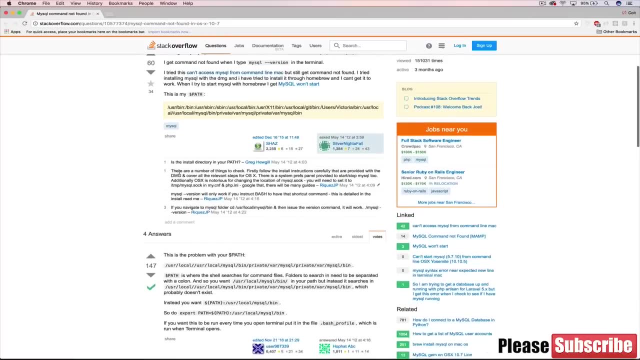 on if you're using bash, and if you are, then you can use a line like this. but essentially you know there's all these possibilities depending on your environment. so i can't cover all of them here, but find the correct command for you to run, and that's only if you're getting command not found, all right. 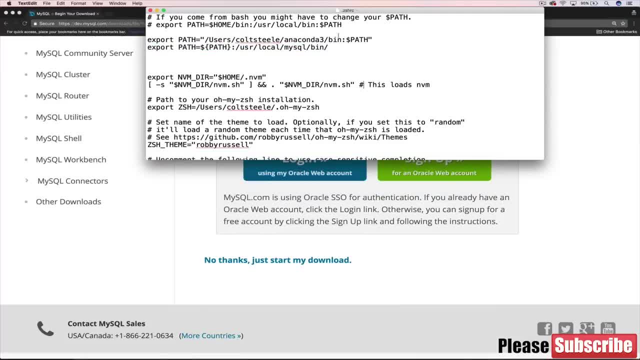 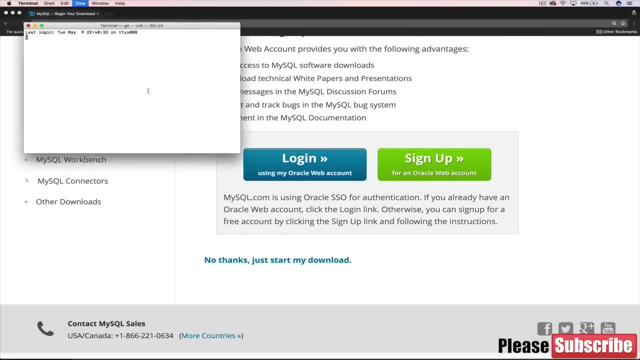 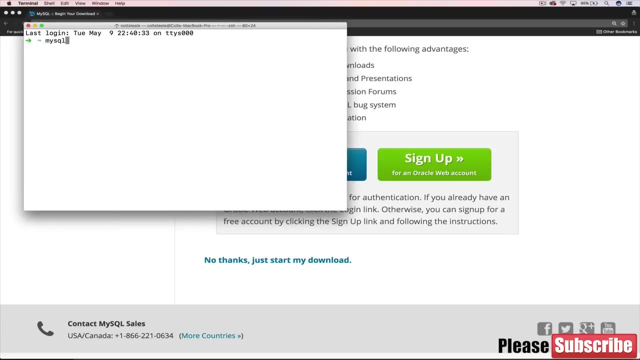 so we need to save this file, close it down, go back to terminal. then the next thing: i'm just going to close the window and reopen it. or you can quit terminal, or you can source your profile. now what i need to do is try mysql again. okay, so now we have a different problem, and this is a 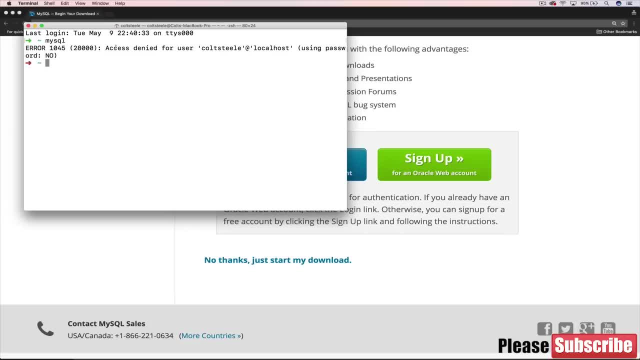 it's not a great problem, but this is the problem. we should have access denied for user colt steel at localhost using password. no, the problem is, if you remember. uh, well, first of all, this means that mysql, the command, is found, it's running, but we're getting a result now, and the problem is that i'm trying to start mysql and i don't. 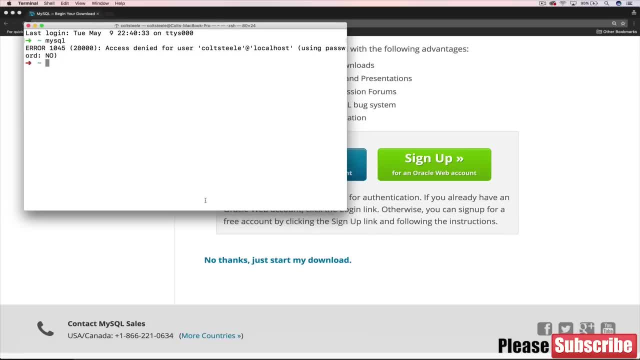 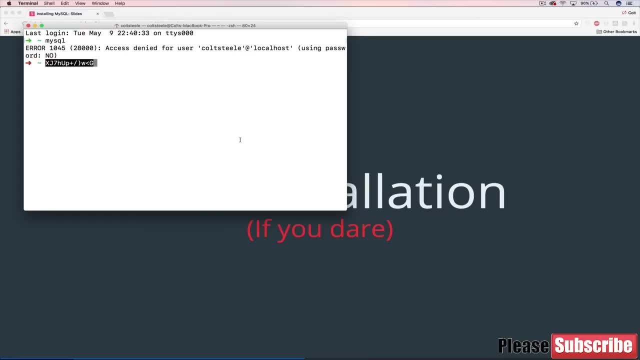 have permission. i need to log in as the root user and remember we saved that password. so i went and copied that password that we were told to save. it's on my clipboard now. i could paste it, but that won't do anything. what we need to do is run mysql dash u, space, root dash p and hit enter. 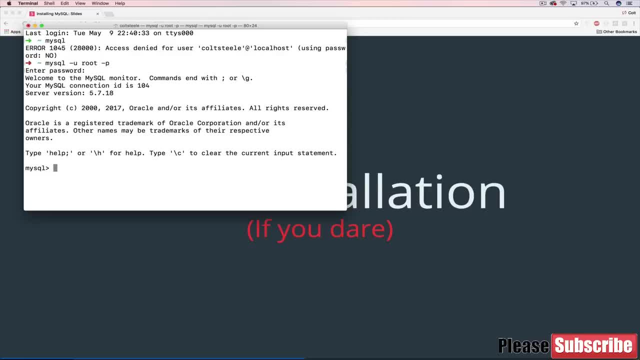 and it should prompt you for the password. you can paste that in and we're in all right. so if you get this far, congratulations, everything's working. if you didn't get to this point, it's likely because of a couple reasons. one is that you're still getting that command. 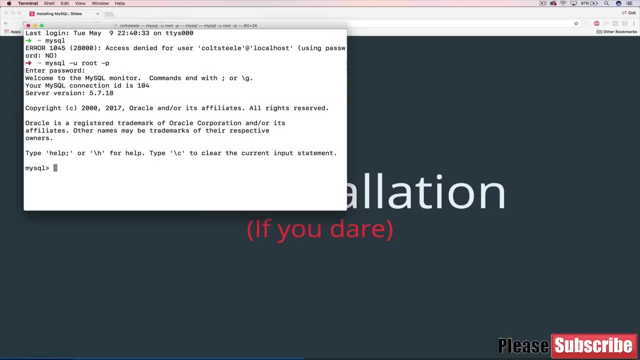 not found issue. that one is is relatively easy to fix. the problem is you have to be comfortable using your command line and opening up, you know, hidden files like bash profile or your rc file. the other problem you could run into is this permissions thing and if you didn't save? 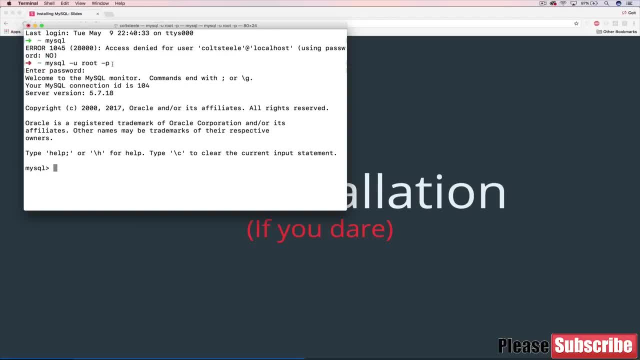 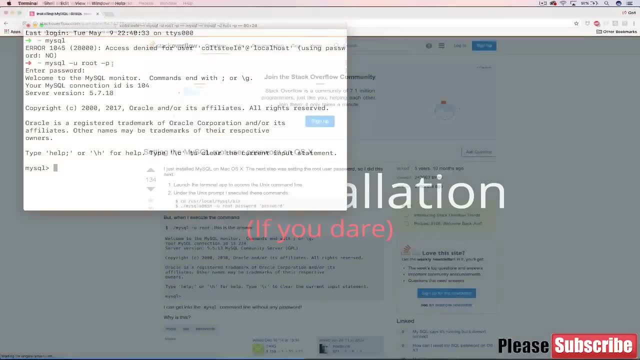 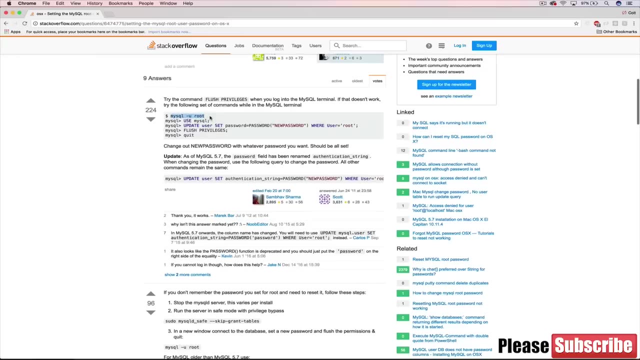 that password that i told you you should save. but if you didn't or you close the window accidentally, you can reset the root password. all you need to do is go online and google it. there's a couple of posts online about it. basically, what you do is you run mysql dash u space root and there's 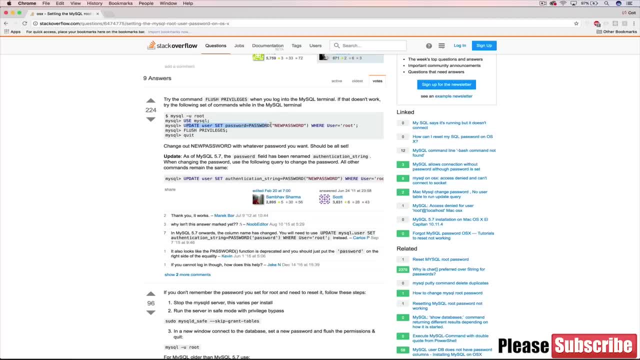 something called flush privileges commands and you can update your password with a new password. there's a couple things you can do like that. basically, rather than me making a video for every possibility, um, it's much better if you just find it out online, and this is why i recommended that. 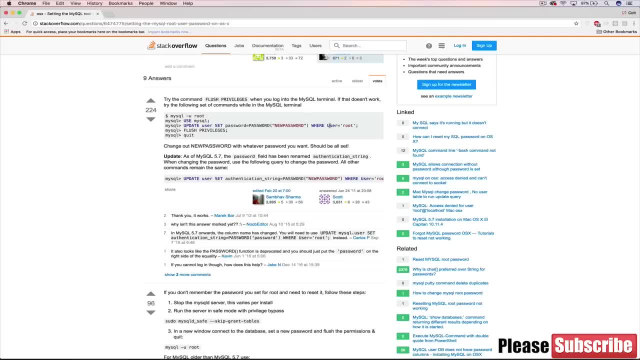 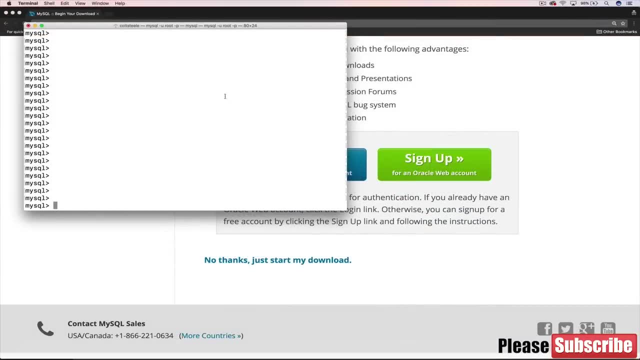 you use cloud9. i promise they're not paying me. it's just that this is difficult, especially in an online setting. okay, so you might think we could start running some mysql code, like, if you tried, here's something we haven't actually seen yet, but if you tried this, or actually, how about show? 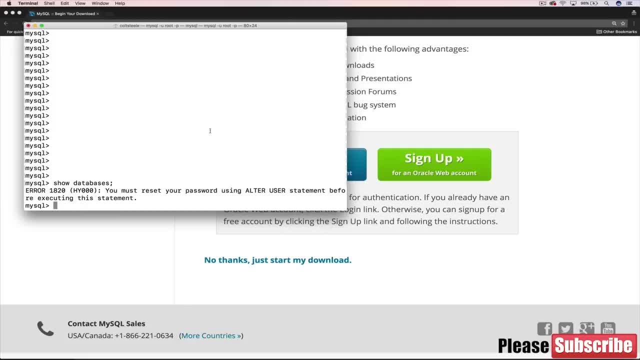 databases. so this would show us a list of databases, and if there are no databases, it should still show us something. but instead we get this: you must reset your password using alter user statement before executing this statement. okay, so our final hurdle here, what we need to do. 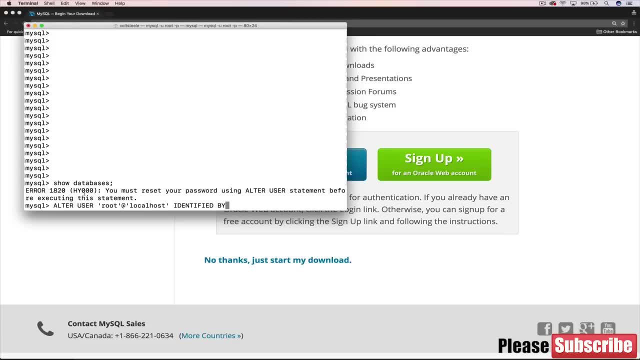 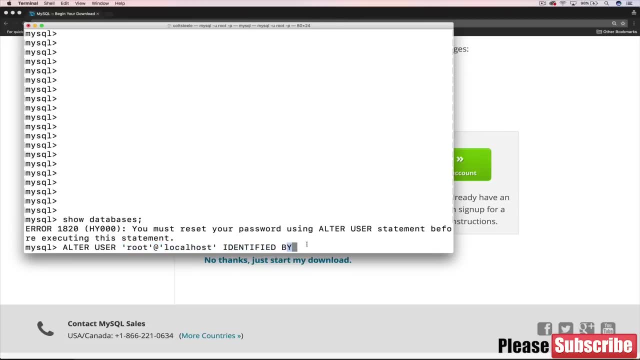 is. i have a command that i just had on my clipboard, but it looks like this: alter user in quotes root at, and then in quotes localhost identified by. and then all you need to do is provide a password that you can use in this case. i'm going to show you how to do that in just a 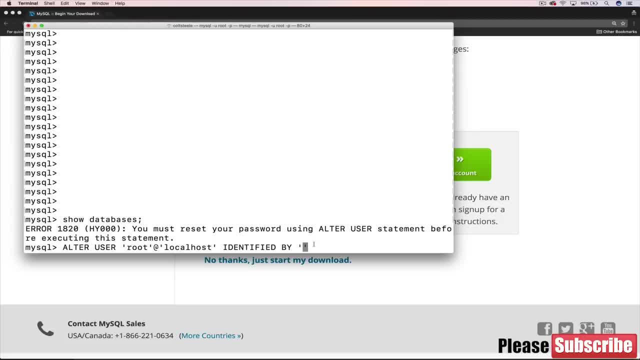 second. so i'm going to show you how to do that in just a second. so i'm going to show you how to do that here in quotes that you would like to use for the root user for your mysql install, for this server instance. and so just type something. i'm just going to make mine password there we go and hit enter. 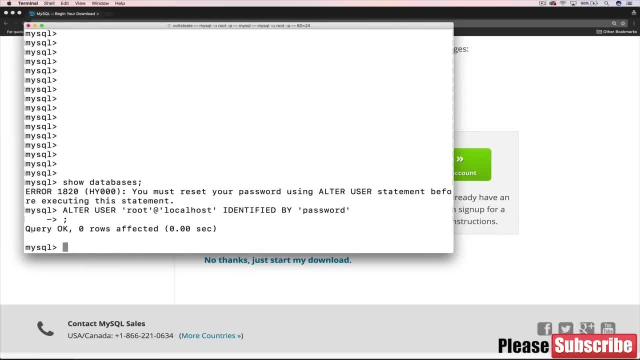 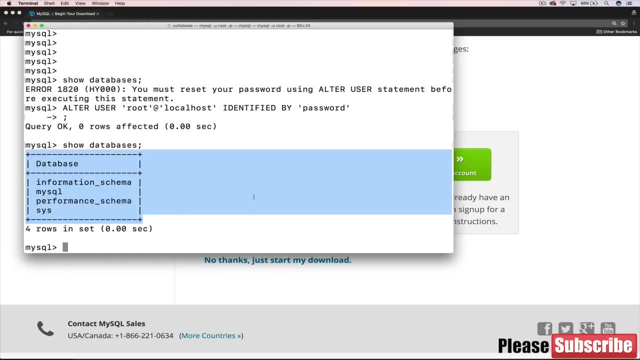 oh, with a semicolon. now, if we get the query, okay, things should be working. if i try my show databases command, this time we're in. i don't get this permissions problem. okay, it worked out. um, so again, that command i'll also include in the instructions if you need to. 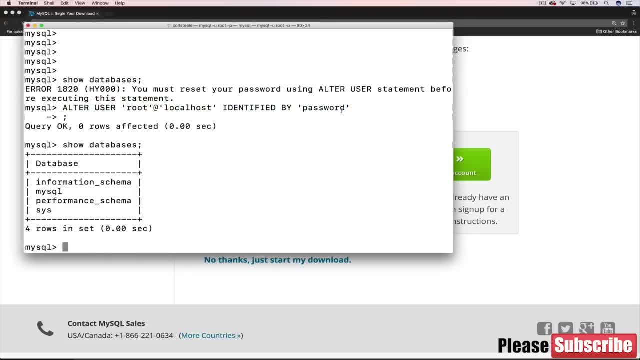 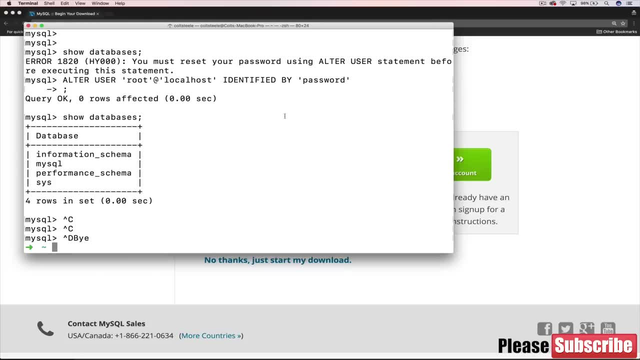 do that. it's just alter user root at localhost, identified by password. okay, so then the last thing is, if you want to close out, by the way, it's command d which we'll be covering all this. if you're going through the course the very first time and this is how you decide to start, we'll 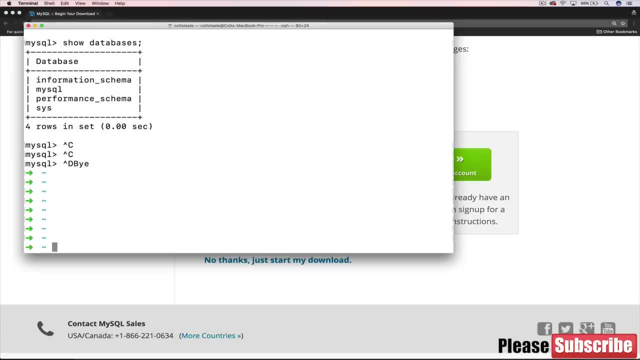 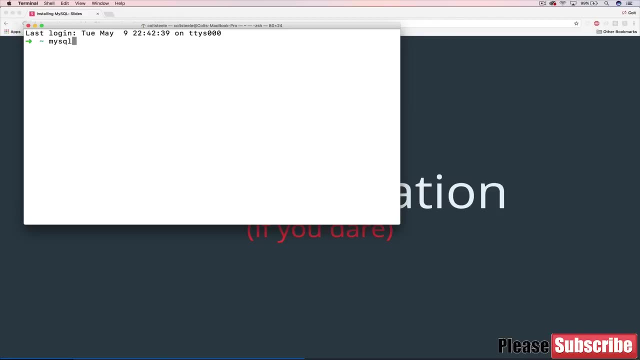 actually go over these commands in the next section when we install everything, or once we have everything installed and we start talking about mysql. but we need to be able to verify the install. so there's a couple commands, okay. so now, if i wanted to try logging in again, i shut it down. it's mysql dash u, root, dash p, and then it will ask me for my. 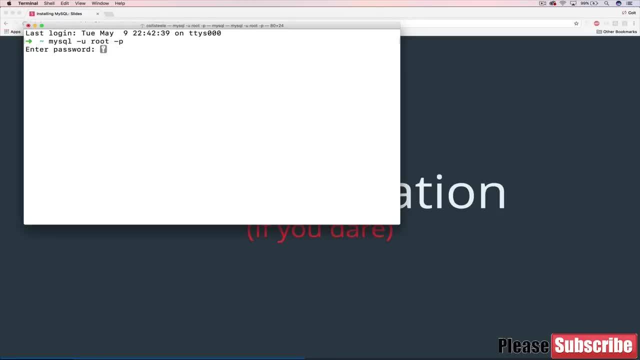 password, which i changed to password, so type that. you won't actually see it, but if you type it correctly, you're in. okay, so that is our journey to installing mysql on a mac. great time. hopefully, if you got to this point, you made it through and everything worked out. 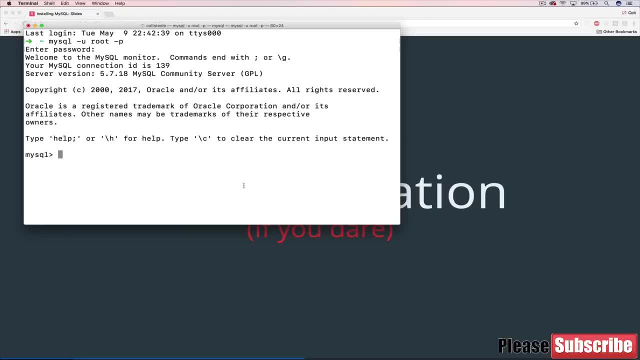 if not, if you're just starting this course off, i still highly recommend that you switch to using cloud 9.. avoid all these issues and then come back to this when you feel more confident. otherwise, if you absolutely have to use a mac, we'll try our best to help you out. 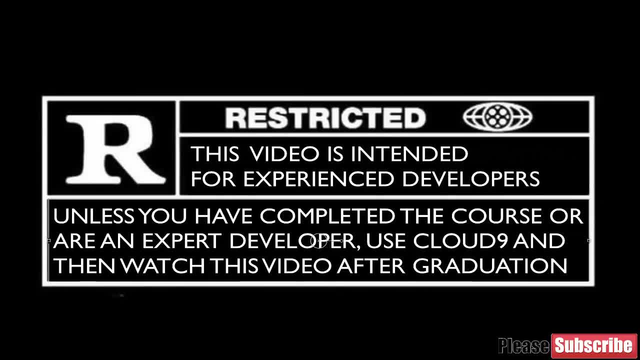 anyways. moving on, warning: this video may contain extremely frustrating installation instructions and is for experienced developers only. it's advised that you install using cloud9 to avoid new software. when you install it, pain and anger. All right, if you're still here after the stern warning, I'll talk about how to. 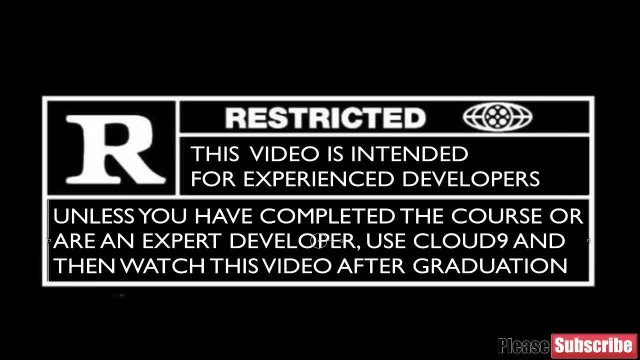 install MySQL on Windows, Of course, remember you will probably run into some sort of issue, depending on your computer and what you have installed already. It can be difficult, So that's why I really, really, really recommend that you use Cloud9.. Skip Windows until the end of the. 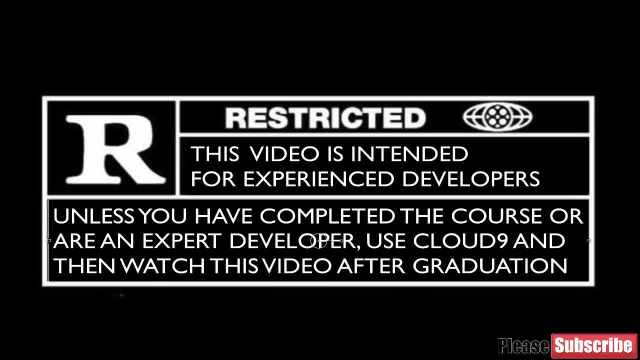 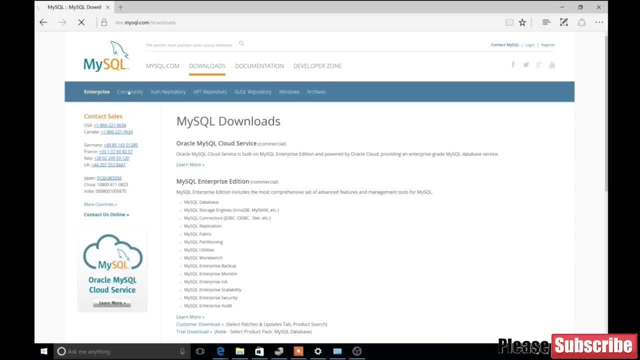 course. Okay, that's enough of a broken record, Let's get started. So to install MySQL on a PC, you need to go to mysqlcom and then click on the download section and then click on community, And under community you can actually click on any of these If you click on download. 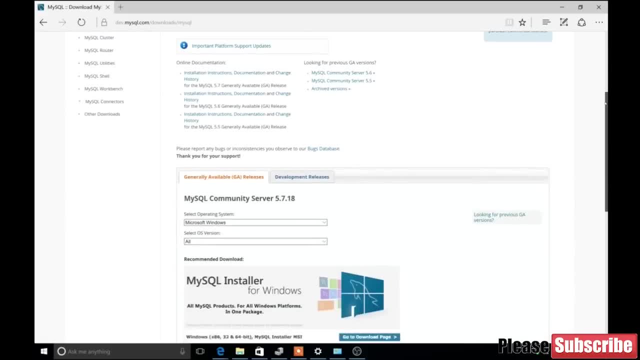 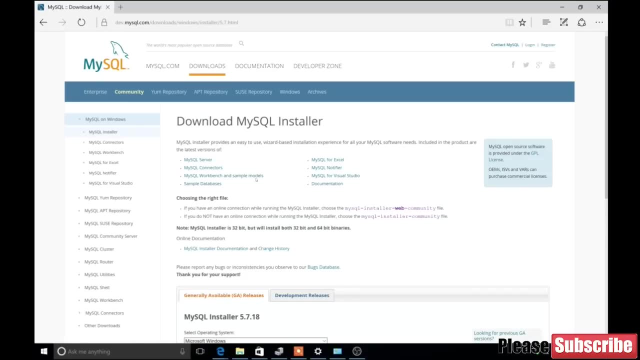 what it's going to suggest for you, if you're a Windows user, is that you actually use the MySQL installer rather than downloading things individually. Basically, it's a package that will help install a bunch of MySQL things all at once that you may or may not use. that you may, or 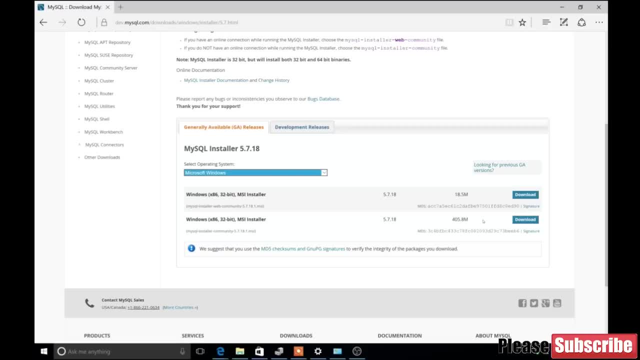 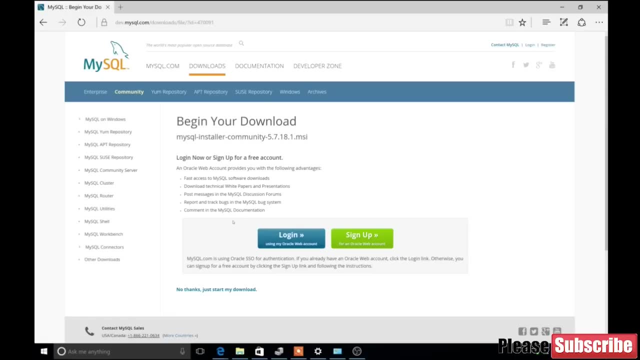 not need. Make sure that you have the correct version selected, depending on your architecture. Then click download And it looks like it starts downloading, but it actually doesn't. You have to click another button at the bottom. No thanks, Just start my download And then I'll fast forward. 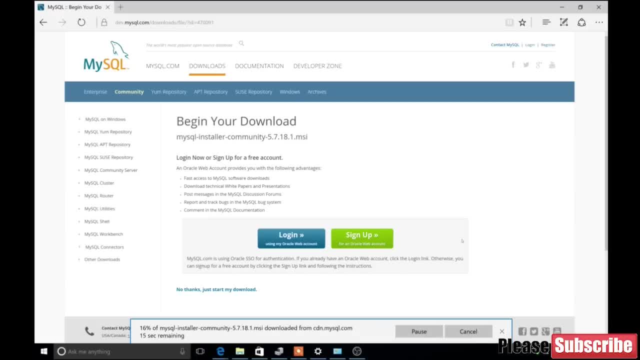 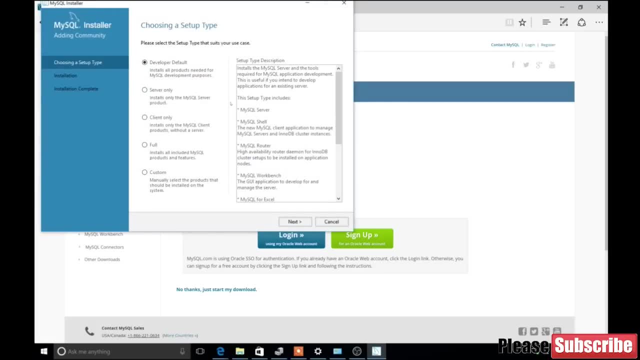 through this. It takes a little bit to download, depending on your internet, But then, once it's done, all we want to do is open it up, run the installer. Okay, so then we have a couple options. We're going to select developer default and then click next And then, depending on what you have, 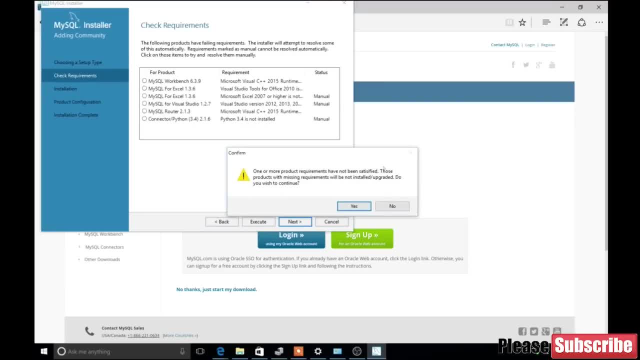 installed on your computer. you may need to actually install some other requirements. So I did here. So I basically had to go through a couple times: double click, click, execute, wait for something else to go, install- in this case Visual C++- And then I had to repeat that a couple of different. 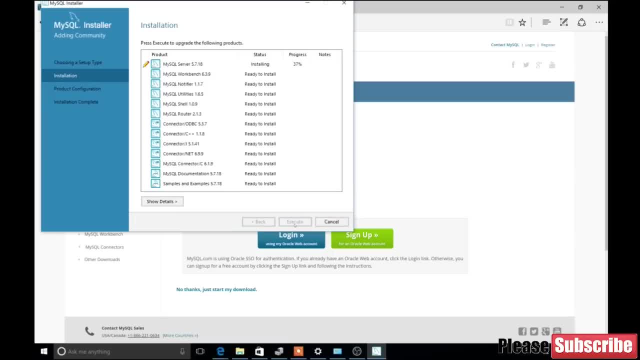 times. Now that will probably be different for you and your machine. But then, once that finishes, click on execute again And this will actually start the installation process. So there's a bunch of components installing, But once they're complete, click next And then we move on to. 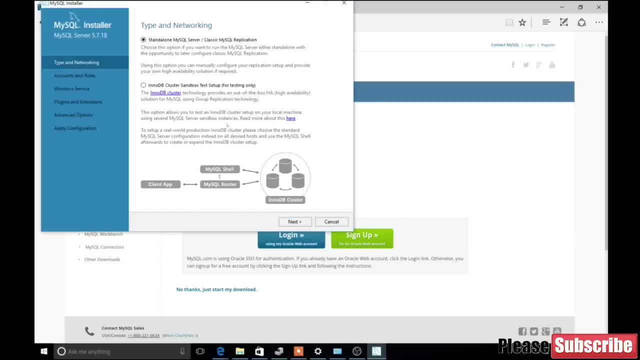 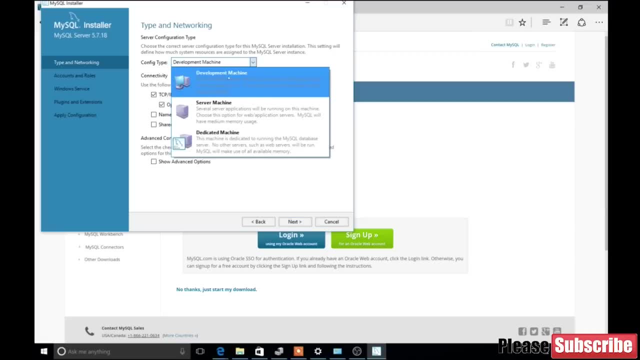 configuration, And all we really care about is configuring the server. So we'll click next again. Basically, click next another time, We don't need to change anything- And further another time, click next. Okay, so we're now at the point where we need to decide on a root password. 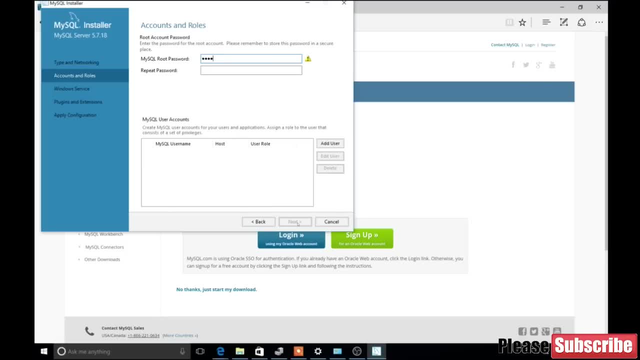 for MySQL, So you can decide on whatever you'd like. I just chose password. the word password It's not a good password, But I wanted to make it simple, easy to remember. So you type it in twice, tells me that it's weak, And then I'm also going to add a user here. You don't have to do this, I'm. 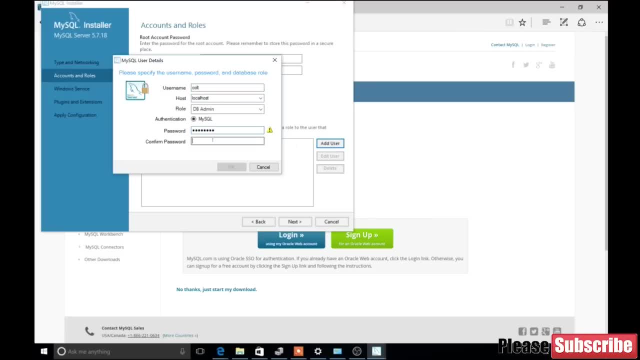 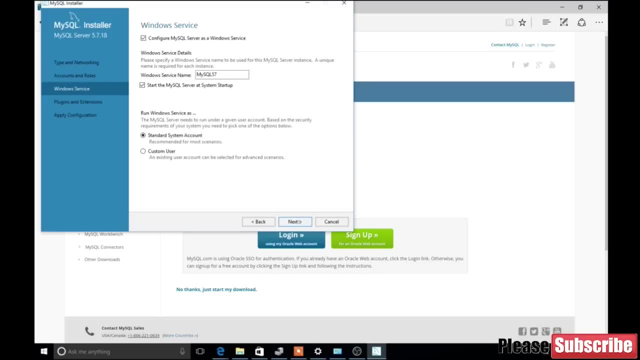 going to make one with the name Colt, And also the password will be password, And then confirm. the password Also tells me that it's weak And I'll click OK. So really all that you need to do is remember whatever password you typed for the root And then click next, And then we'll click. 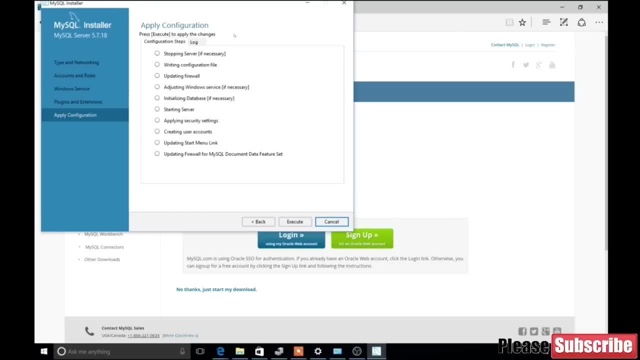 next one more time And then, finally again, we'll click execute And it will start to apply the configuration And it may take a moment or two, But then, once it finishes, everything should be installed. So we'll click finish and then get out of here. So that's how we install. 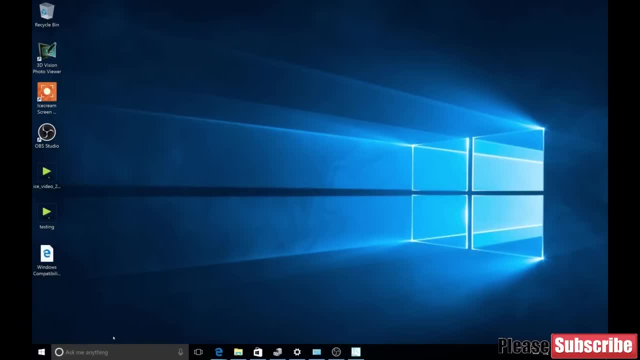 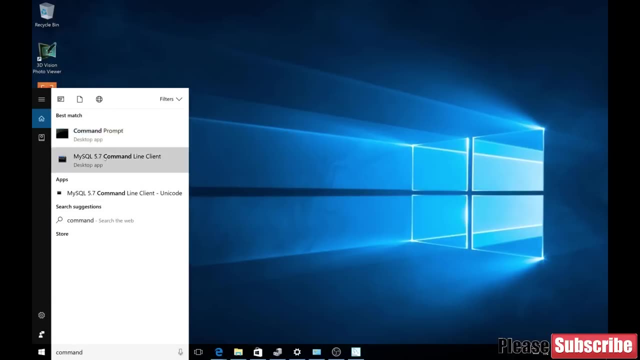 the next important thing is starting up the command line client, which you can find just under MySQL command line client. Click on it, And then you'll need to enter your root password, which in my case was password, And now we're able to actually type some code, something like show: 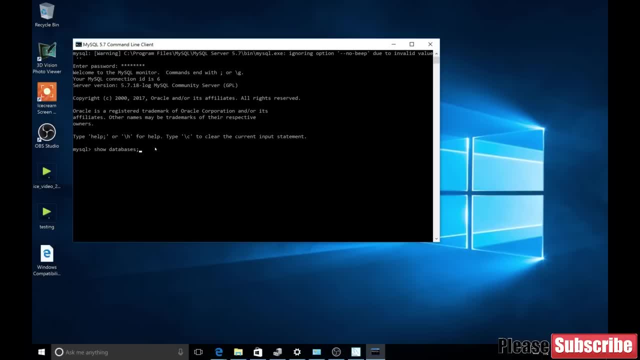 databases, which we haven't talked about, But you can type code in there. You can also try typing things that aren't SQL And you'll see you get error messages. But all that we really need to care about is that we have the command line client up and running and we can type stuff into it. 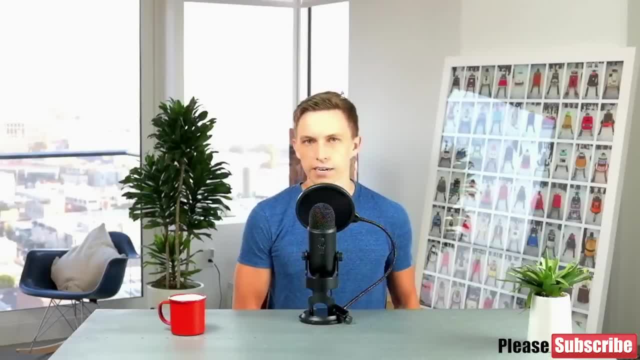 So let's go back to another one of these videos. This time we are diving into section three, a really important section, And yes, you could probably say that about everything in this course, But this is where we really get going. It's really crucial In the last section, it's true. 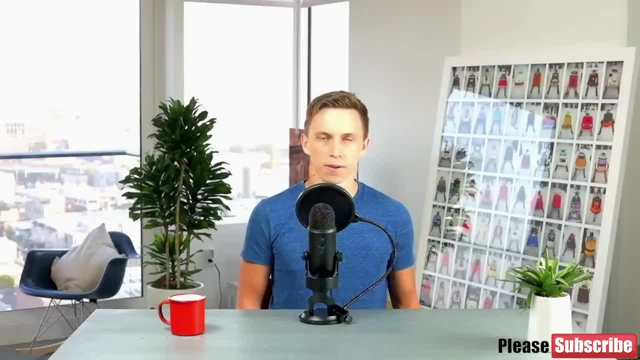 we did run our first MySQL commands But if we're being honest, they're a little bit underwhelming, kind of lame. they didn't do much In this section that actually changes. we see our first commands around data, So we'll be able to make a new database or delete a database And then inside of 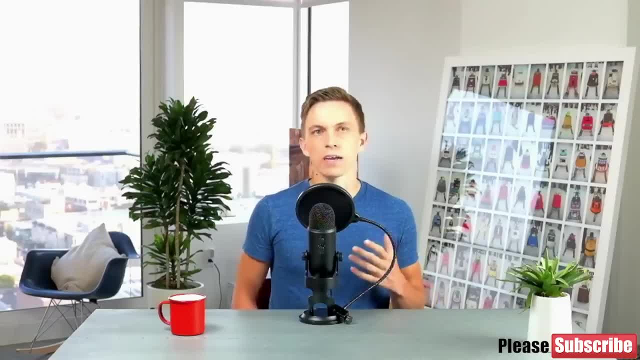 those databases. we'll start working with tables, which are kind of the fundamental structure in all of SQL and MySQL. So really important stuff, And by the end of the section we'll actually throughout the entire section are sprinkled a bunch of exercises around commands that we'll. 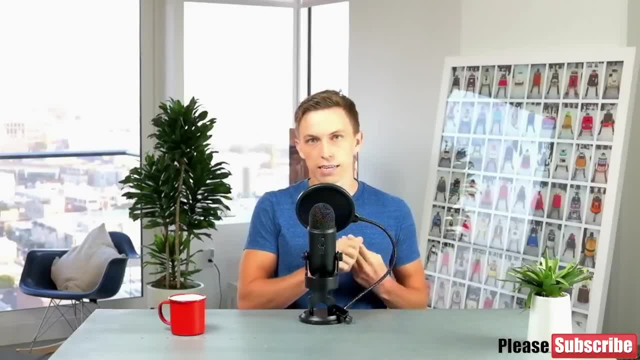 learn things like creating databases, using and switching to databases and then creating tables and describing tables. So a bunch of challenges coming up. But, like I said, this is a really important turning point where we actually get past all the garbage around setting stuff up, installing. Now we're actually doing real MySQL stuff, So let's. 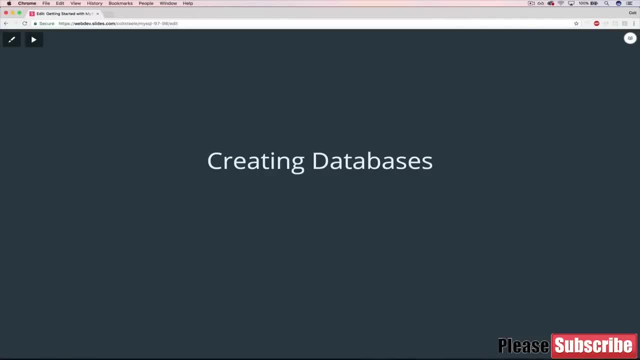 get going. Okay, so in this video we're going to talk about how you actually create new databases in MySQL Finally. So before we go into the code, let's set the stage just a little bit. Currently, we have a MySQL database server, represented by this box that's running on our Cloud9 instance. 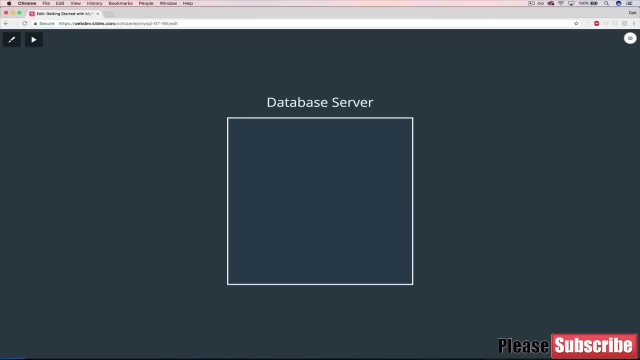 So that's what happened when we did the MySQL dash CTL start. that started up the database server. So now the command that I'm going to show you is what allows us to create individual databases inside of the MySQL database server. So, hypothetically, we could have a database for a dog walking app, Another one for a soap shop. We 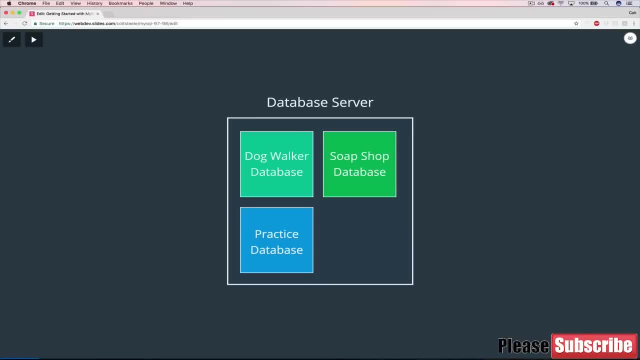 could have a practice database. If you were just practicing some new codes and new lines of SQL, you would probably have a database for dog walking And maybe there's a news site database And they're all hosted. they're all part of the same database server But their individual databases. 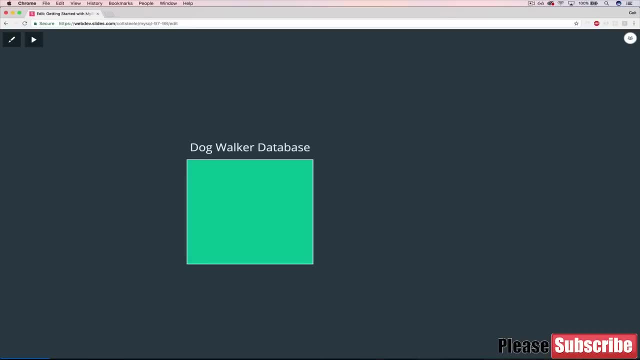 inside And that's really important. And to understand why, let's zoom in a little bit on two of the databases: our dog walking app database and a soap shop database. So inside of those two databases we'll store various entities or different data. So in the dog walking database, 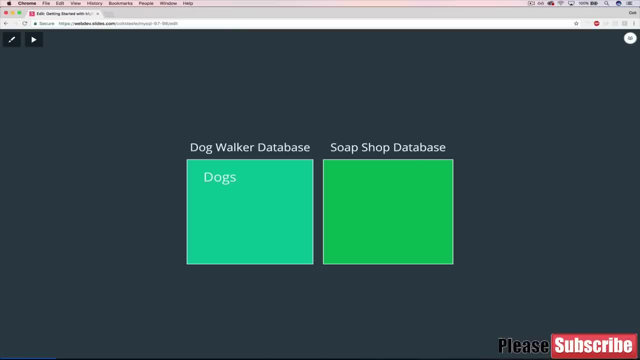 we'll probably need to store information about dogs, And in our Soap Shop database we'll need to store something about soaps. And then here's where it gets really important. Our dog walking app likely has users, but so does our Soap Shop app. 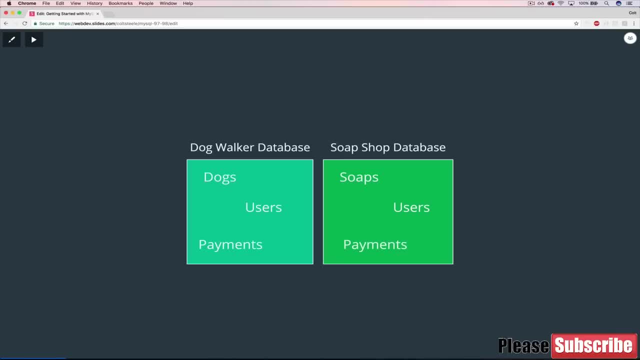 And our dog walking app has payments and so does our Soap Shop app, So they have to be separated. If we just had one database that everything was using on this server, there would be a lot of crossover and there would be issues. But if you had somebody who had the same name, who used your dog walking app, and they also- 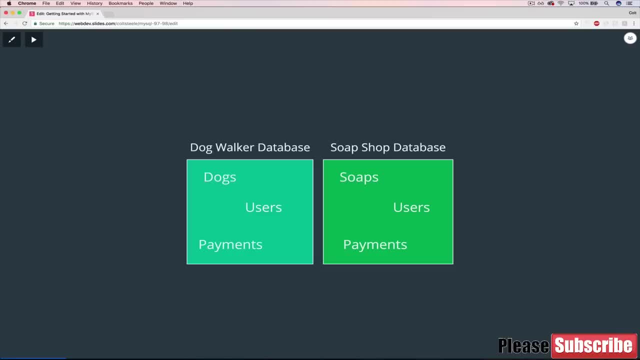 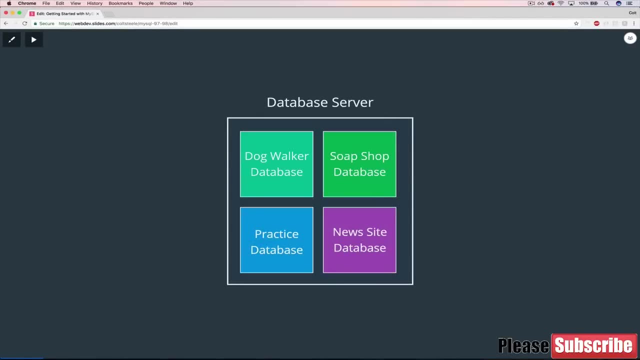 used the Soap Shop app and the streams got crossed. if you will, that's problematic. So what we're going to learn now is how to create these individual walled-off databases inside of the MySQL server we have running. Okay, so let's take a look at some code. 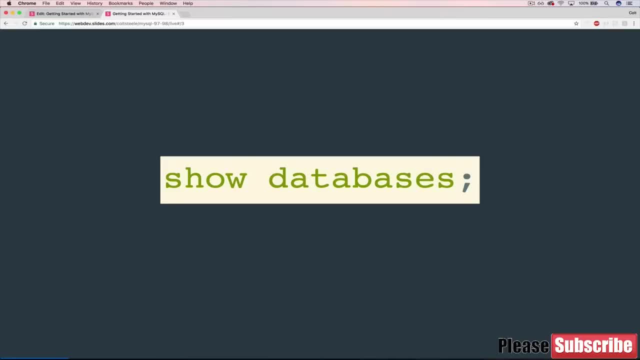 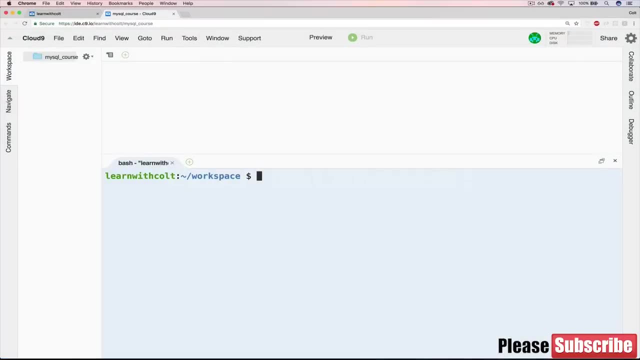 This first line here we've already seen before. All that it does is list the current databases that exist in the MySQL server. So when we do it right now, I need to start up MySQL, CTL, CLI and I type show databases. 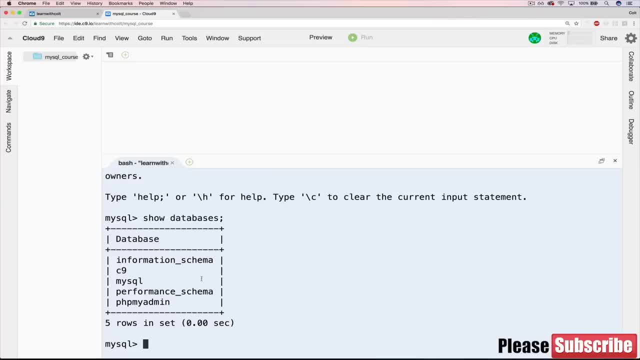 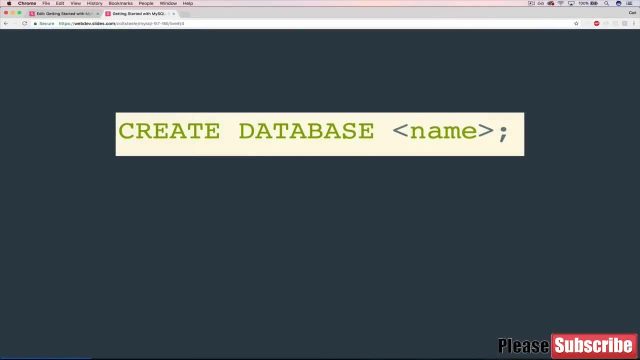 We get this list of the five pre-existing ones that we have nothing to do with. We didn't create these manually. The next piece of code is create database, followed by the name of the database you'd like to create. So, in this course, whenever there's a variable, I'll use these brackets to signify that. 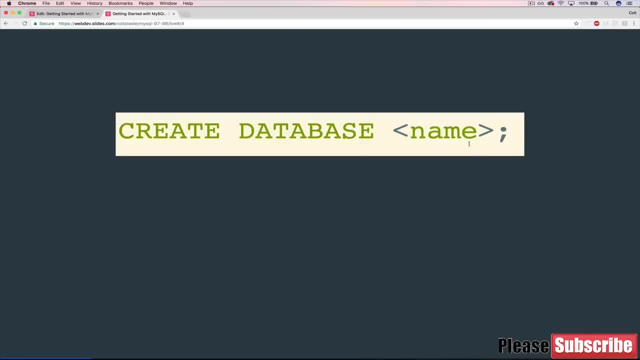 it's just a placeholder. So in this case, whatever the name of your database is, and then a semicolon, So to make a database for our Soap Store, we might name it soap underscore store. Or for our dog app, we could use dog app and you don't have to use underscores. 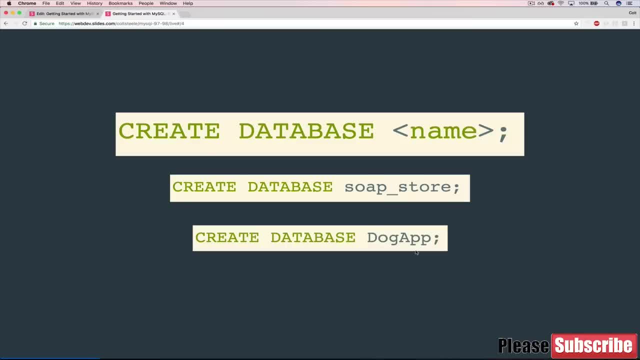 You can capitalize things if you would like. There's no rules governing that exactly. However, if you did something like this, while it can work, it's just not a good idea to do it, So that gets X'd out. I don't recommend doing it. 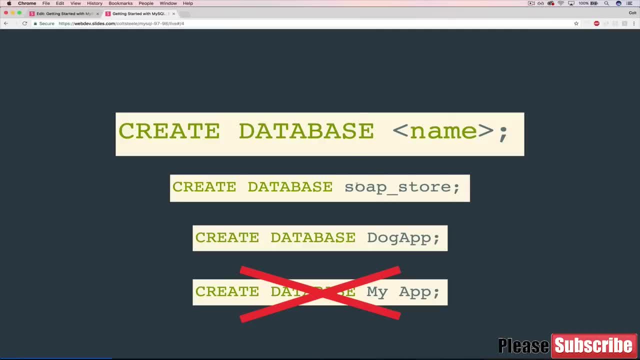 Actually, my recommendation is to stick with this here, what's called snake case: Everything's lowercase and just use underscores instead of spaces. But it's totally up to you. Like I said, there's not a hard rule And what's more important is that you are just consistent. 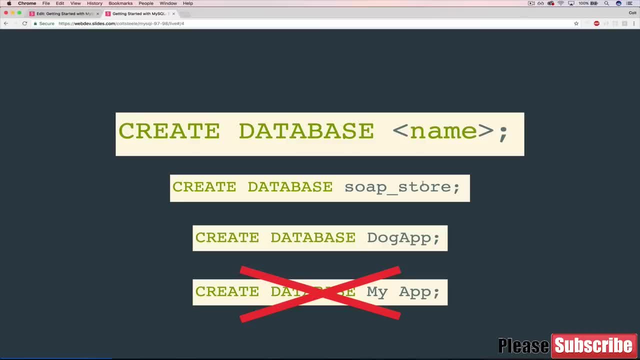 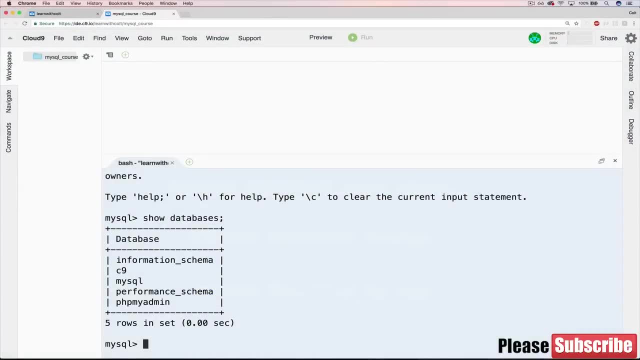 So, whatever you choose, just make sure that you continue to use that, just to avoid any confusion. So let's hop over to our terminal and give it a shot. So I'm going to just make my first database And I will call it hello world DB. 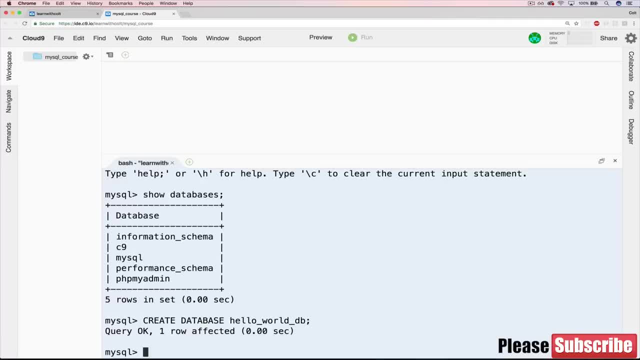 And remember that semicolon. And if we wanted to make sure that it worked, we can just run that show databases command again. Now you'll see a new addition. hello world DB. A note about capitalization When I wrote create database. 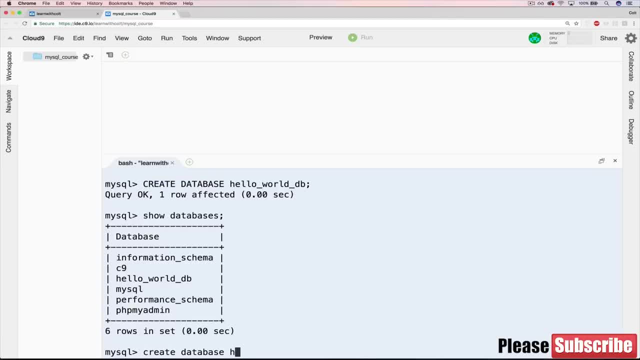 Yes, I went away with doing create database, Hello, and let's call this one testing DB. That works just fine. So whenever you see those capitalized letters in SQL commands, you do not have to use them, But I like to use them and a lot of people like to use them just to signify what comes. 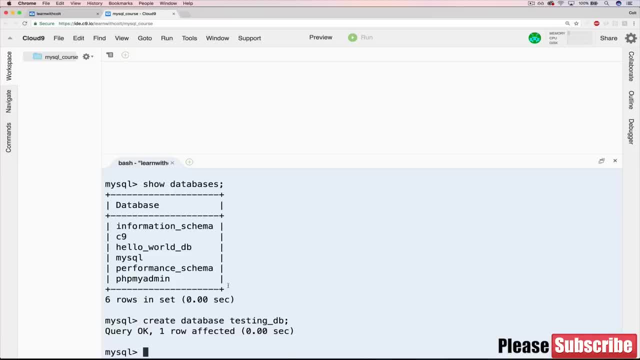 from SQL and then what is a custom name? So in this case, testing DB is something I wrote, or hello world DB is a database name or a table name down the line or a column name once we get there And we can tell that, because it's not capitalized. 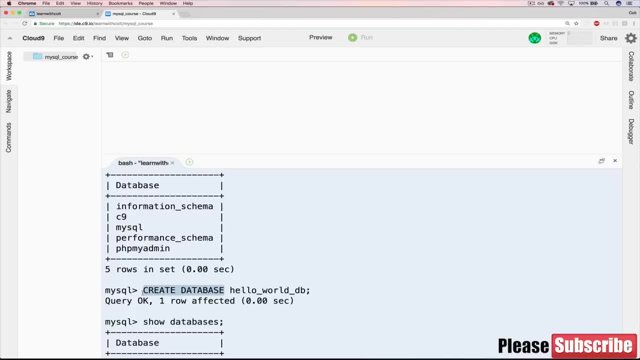 And then create database is in all caps. tells us that's just regular old SQL. Okay, so that's pretty much it to creating a database. that doesn't really give us very much, but we've basically made a space on the server where we can add data. 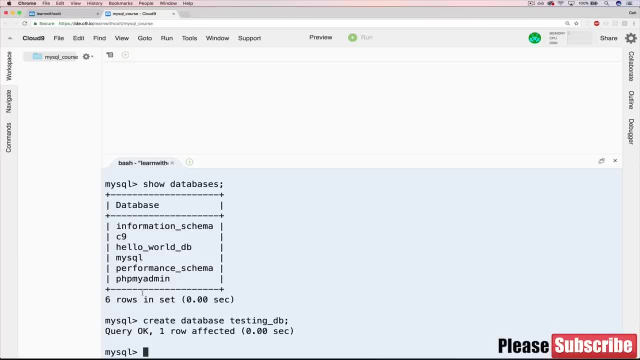 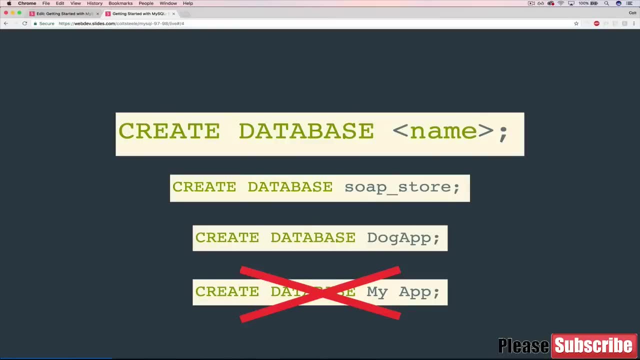 We just don't know how to do that yet. So we've just partitioned off a little area And we've given it a name of hello world DB Or, in our second example, testing DB. So we've seen how to create a database. 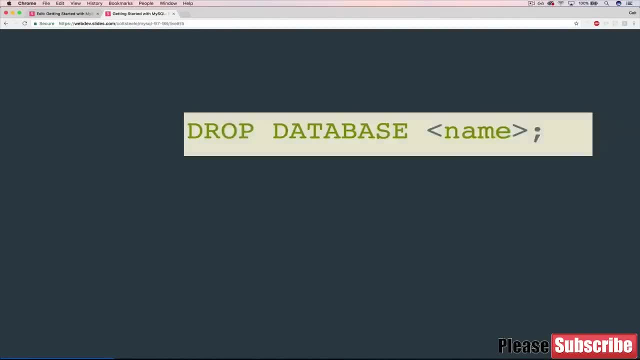 And the natural next step is to see how to delete one. It's pretty simple. The command is drop database and then whatever the name of the database is that you're looking to delete. So we'll come across this term drop here a couple of times in the course. 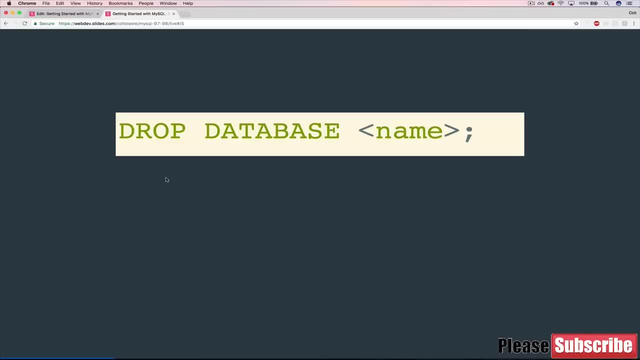 It's basically the SQL version of delete, and we'll be able to use it to drop things other than just a database, Be able to delete Tables, for instance, once we get there. So let's try it out Back in cloud nine. 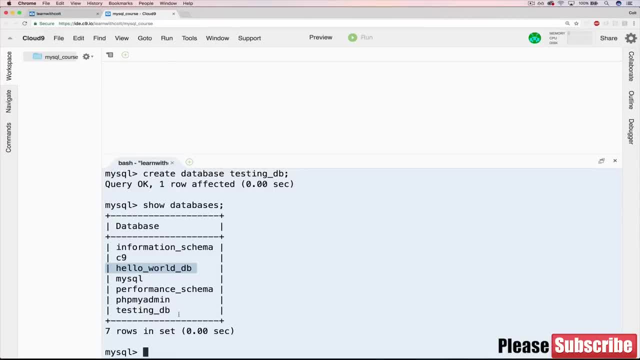 When I ran show databases, here are two that I created. I'm not going to delete any of the pre-existing ones, I just don't want to mess with that. So we will delete both of these though. Hello world DB and testing DB. 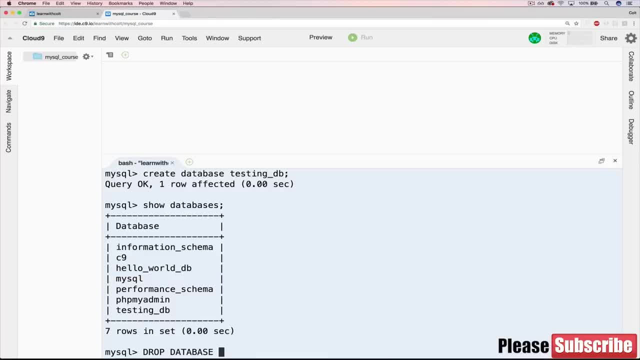 So let's do that now: Drop database, Hello world DB, Semicolon. And you can tell that it works, first of all because it said query OK, But then also, if I recall, show databases. This time hello world DB is gone. 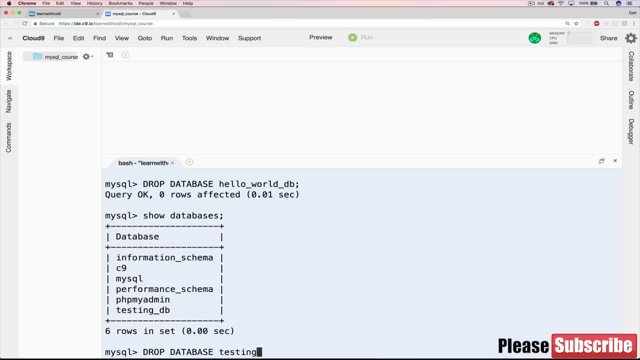 Let's do the same thing: Drop database for testing DB. This time I'm going to leave off a semicolon, not because it's a good idea, but just to remind you that your code will not execute until you add that in there. 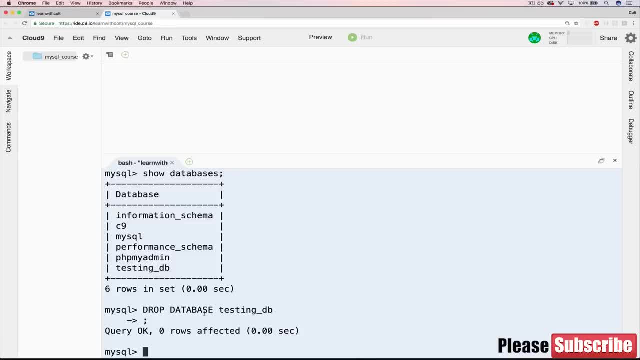 It doesn't matter that it's on a separate line. We'll be writing multi-line queries, just a little bit. What does matter is that it's there at all. It's what indicates that you're done and that it should run. So we can just double check that it worked. 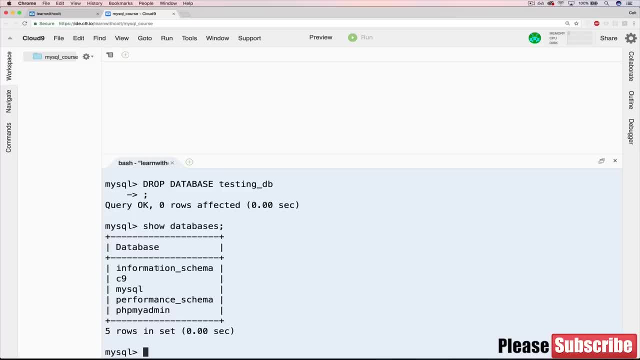 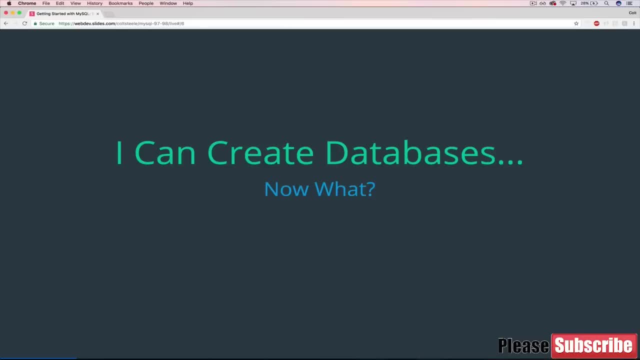 Now our testing DB is gone as well. So that's all there is to dropping a database. Pretty straightforward command, All right. So we saw how we can create databases and destroy them. So what comes next? We're going to see how we actually use them. 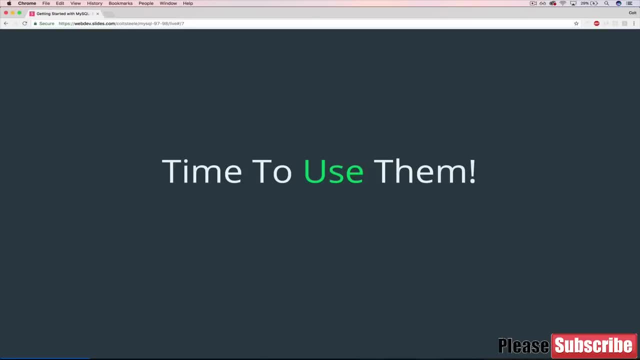 And I mean that in a very literal sense. In MySQL there is a use command And what this does is it tells MySQL which database we want to be working with. So we have potentially 10 different databases on one MySQL server and we want to search. 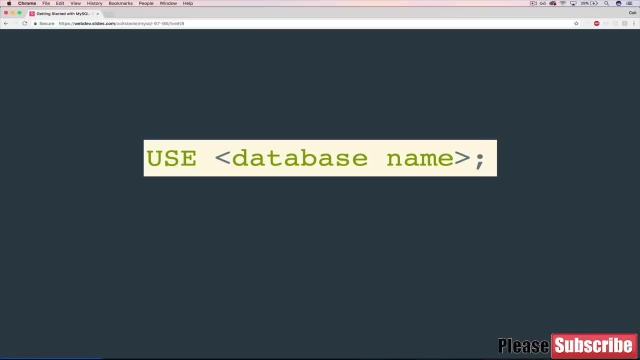 some data from one of them. Well, we need to tell MySQL which one we want to be using at any given time, And we can switch between them using the use command that you see right now. So we're going to use the use command that you see right here. 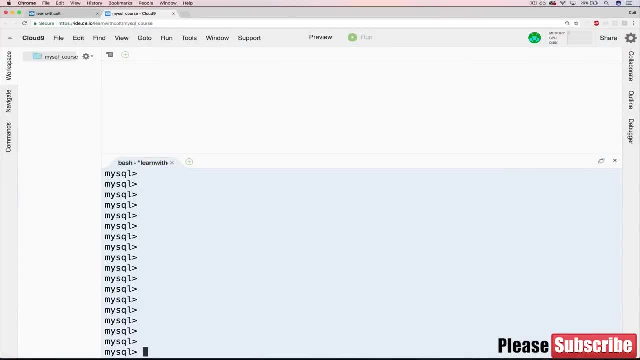 So I'll really quickly show you how it works over in Cloud9.. So if we create a new database and we'll just call this one dog walking app And we hit Enter, We do show databases. There it is, And if I want to use that, all I have to do is type: use dog walking app. 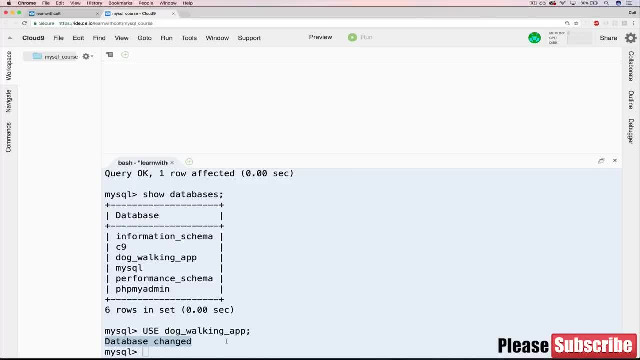 And then save the database And I'll click OK. We don't see much except for database changed. That's a good thing, But if we wanted to know for sure what database we are currently using, there's another MySQL command that we can use. 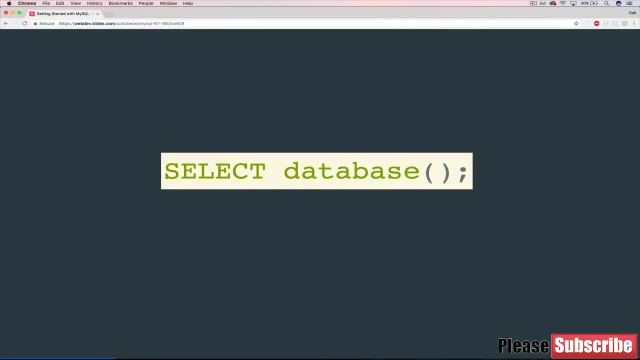 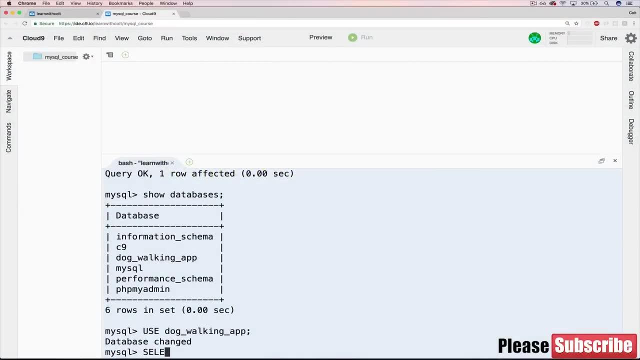 And that command looks like this select database, with parentheses after it, And what this will do is tell you the currently used database. So let's try that out Back in Cloud9, if I type select database with those parentheses and a semicolon, it 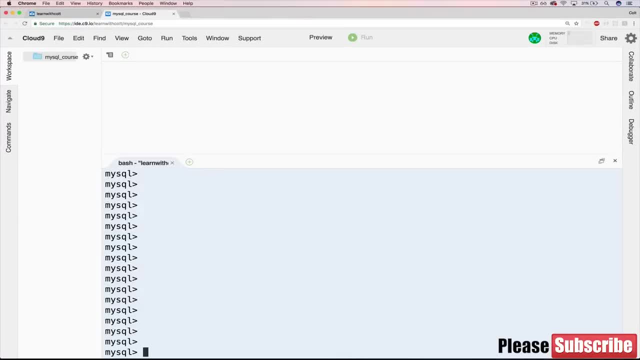 tells you. tells me database is dog walking app and if I decided to delete that database I would use the drop database dog walking app command. it tells me: query. okay, I do show databases and it should be gone. but if I do my select database command, pause and think to yourself for a moment what database 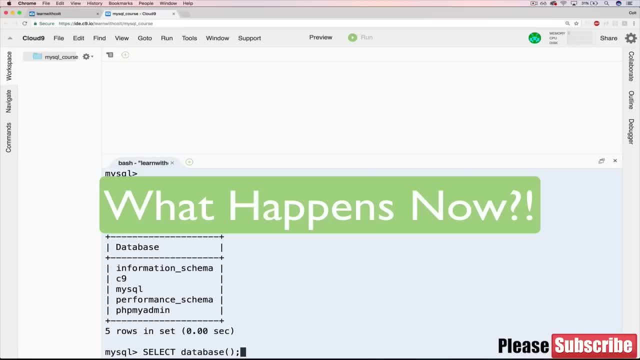 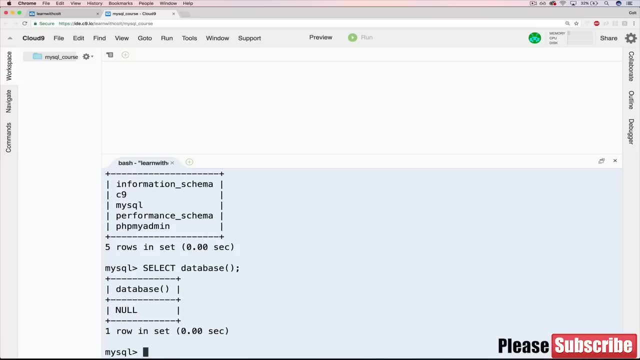 do you think I'll be using right now? we were using the dog walking app, but then we deleted it. so now what? and here's the answer- kind of a trick question: we're not using a database right now, hence the null here, and we'll be talking a bit more about null throughout this course. but 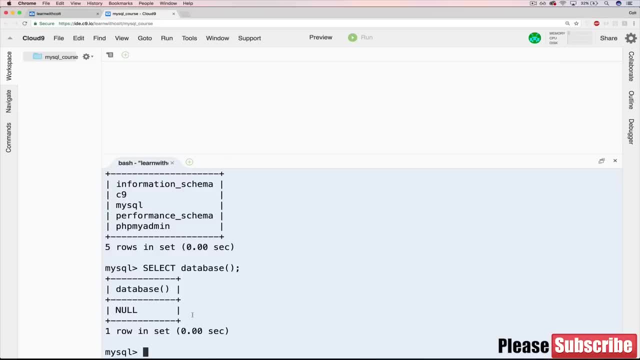 that basically means we're not using any database. so just to show you one more time if we switch. let's say I wanted to use one of these pre-existing ones, like the c9 database. I'm going to use the c9 database and I'm going to use the c9 database and I'm going to use the. 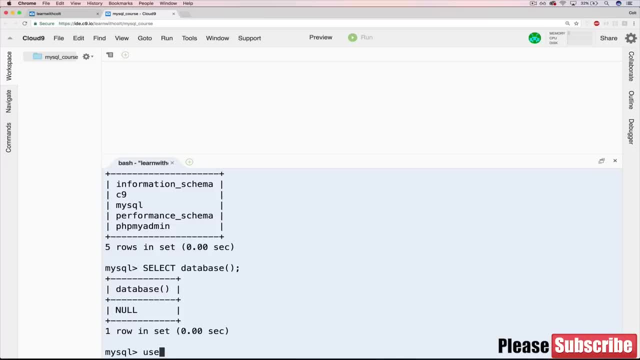 I'm not going to delete that, but if I wanted to, I just use c9 and now, if I do, my select database tells me database is c9. okay, so that's all there is to using a database and then also this select database command to see your current database next up. we'll start talking about tables and putting. 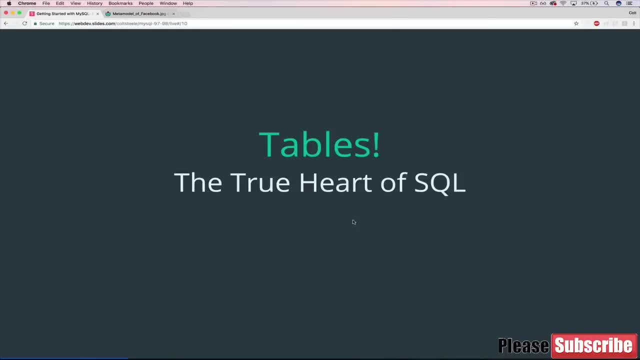 some data in these databases as soon as possible. so the next couple of videos are all about tables, which are the most important part of sql. they are the true heart of using sql and in this first video we'll start off by setting the stage or setting the table. if you will, let me get away. 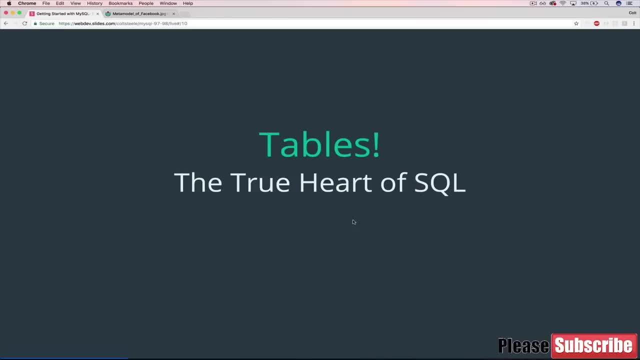 with that for how they work, what they are, and then we'll dive into data types next, and then we'll actually create tables and see the code that you use to create them. so let's get started. the first thing you should know is that a database is just a bunch of tables. so we've already gone and 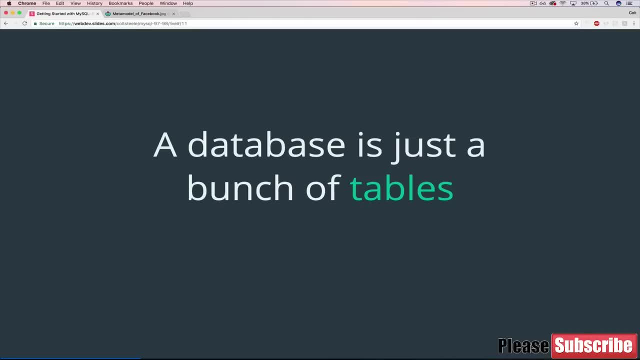 created a couple of empty databases and deleted them as well, but what goes in them are just a bunch of tables. That's where the data is stored. As a short aside, this is in a relational database, so everything we're talking about that uses SQL- things like MySQL, Postgres, SQLite, those are. 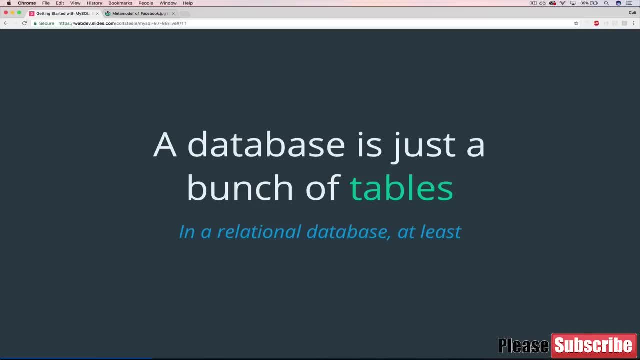 relational databases and they use tables, They use tabular data, but not every single database in the world does, and we'll see some examples of those later on. This course is not about those types of databases, but it helps to kind of bring them in, to show you some contrast to what you're. 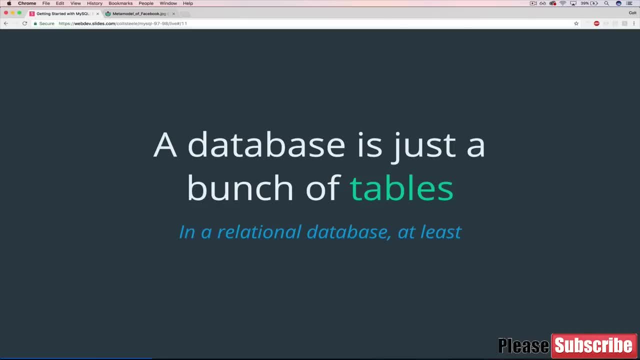 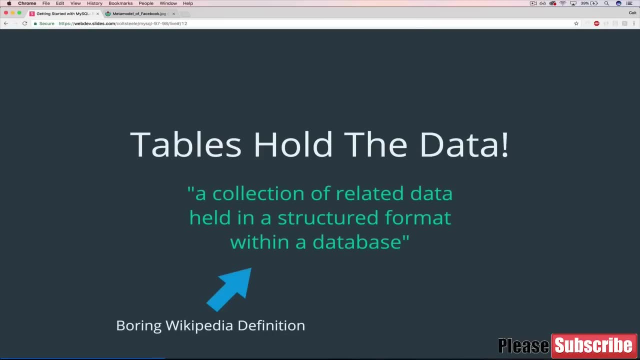 learning, so we'll see that later on. Just a short caveat there. So tables hold the data. That's my definition. If you want the boring Wikipedia definition, it looks like this: Tables are a collection of related data held in a structured format within a database. Hopefully you're still. 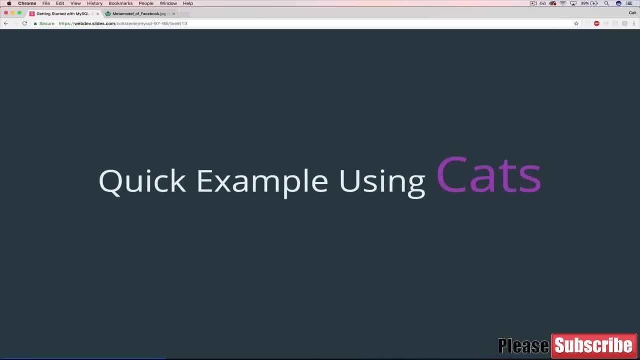 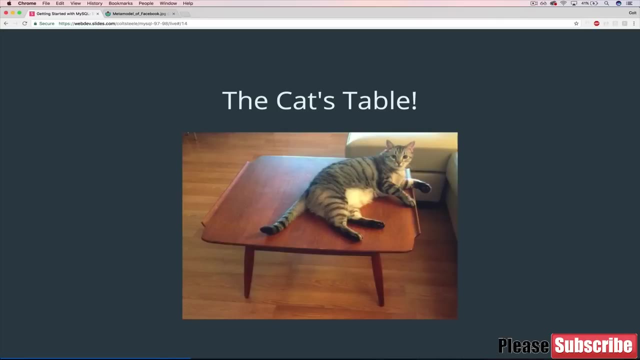 awake after that. But let's take a quick example using cats. So we're going to model some cats data using a table, Okay, so let's take a quick look at the cats table. Drum roll please. I know it's pretty hilarious. You're probably falling out of your chair. 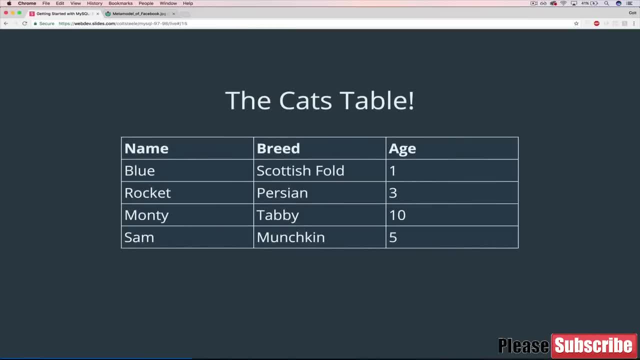 All right. so the real cats table, at least in this context, doesn't have an apostrophe. looks something like this, And of course, there's a million different types of cats in this table. So let's take a quick look at the cats table. 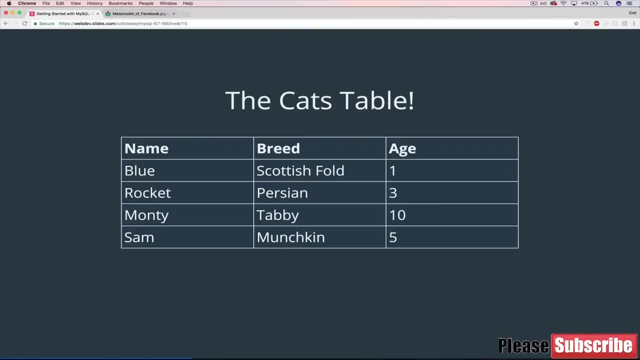 There's a million different ways we could break down the data for a cat, for modeling cats. In my case, I just went with name, breed and age. So we could do plenty of other things like location, gender, is spayed, is neutered, that sort of thing, but just doing name, breed and age. 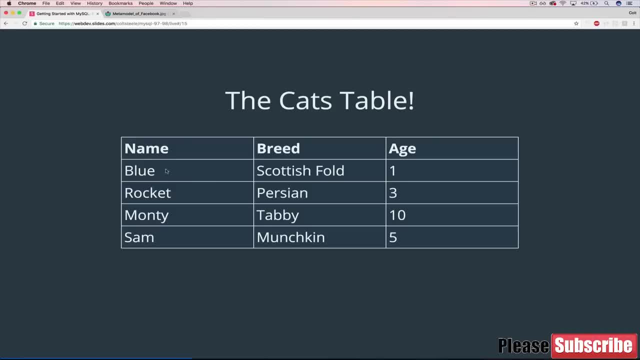 So I've put a couple of cats in here. We've got Blue, who's a Scottish Fold, who's one year old. That's my cat. We've got Rocket, Who is a Persian, who's three years old. Totally made up. 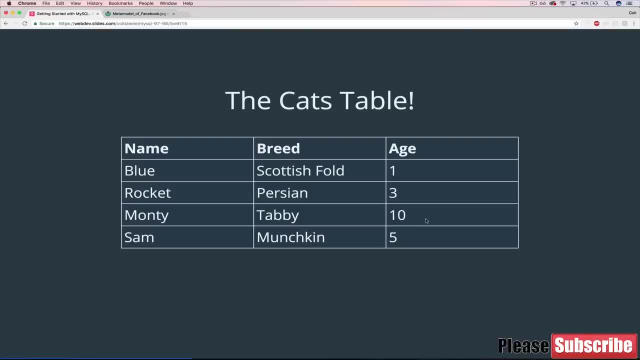 Monty, who's a Tabby, who's 10 years old. That is my childhood cat. He's still kicking and biting people. We've got Sam, who is a Munchkin, If you don't know what that breed is. 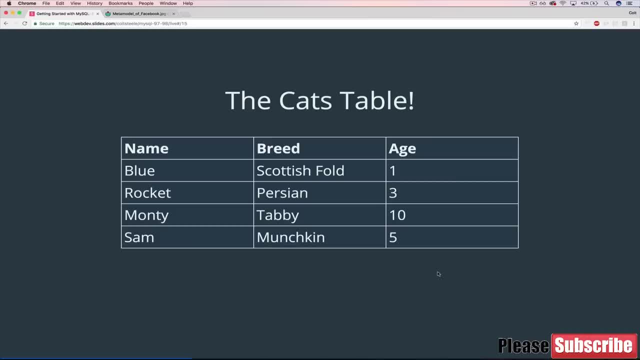 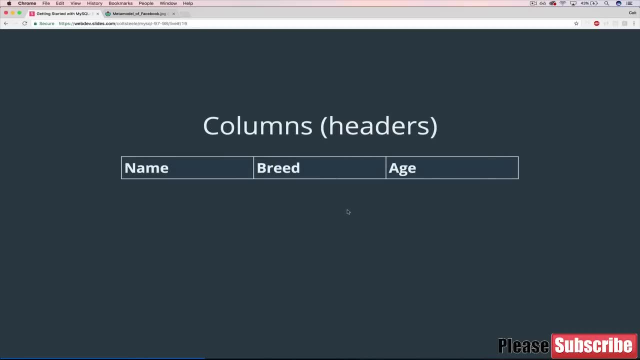 look them up. They're pretty hilarious, although kind of sad. They have really stubby legs. Who is five years old, Also made that cat up. So some terminology: When we're talking about tables and you hear the term columns, it's referring to the headers on that table. So what are the different components of data? 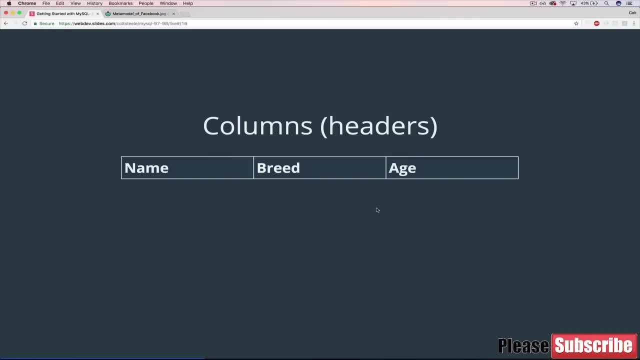 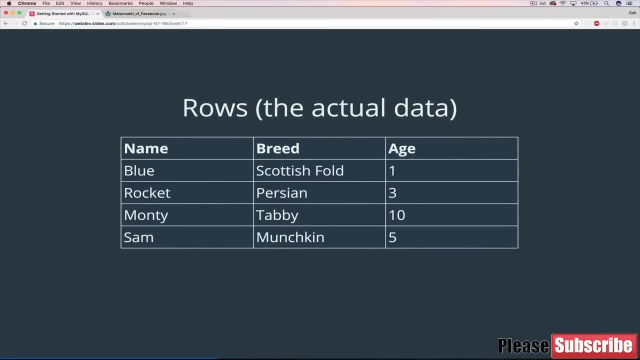 the different pieces that have to be there. In our case we have name, breed and age, So those are the columns, and then the rows are the actual data in the table. So here's a row: Blue, the cat is one row. Rocket is another row. Monty is another row. Sam is another row. 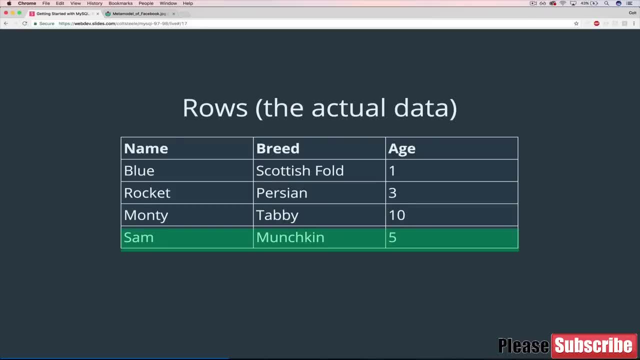 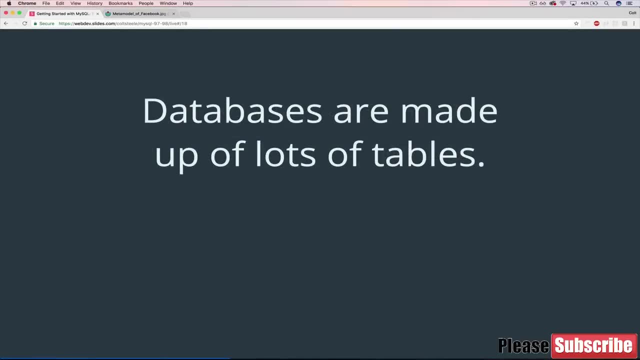 I really wish those lined up correctly, but I just drove myself nuts trying to get them all together, Please forgive me. Anyways, so databases are made up of lots and lots of these tables. It's usually not just one If you have a really, really simple app and you're just storing one. 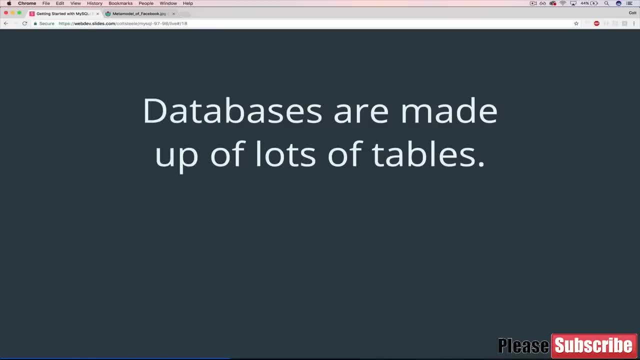 thing, then it will just be one, But usually apps are pretty complicated and data is complicated. All that we modeled there was cats, but imagine if this was actually an app. Let's say it was a pet sitting app and cats were one thing that we had to keep track of. but we also have to keep 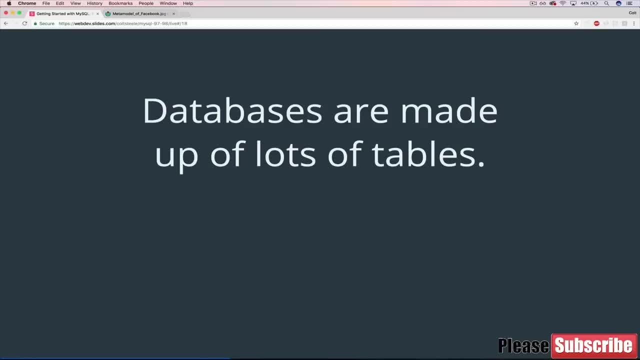 track of cats. So we have to keep track of cats. So we have to keep track of cats. So we have to keep track of owners and the pet sitters and addresses and dates and appointments and payments, and those are all going to be tables. Some of them might even be multiple tables. 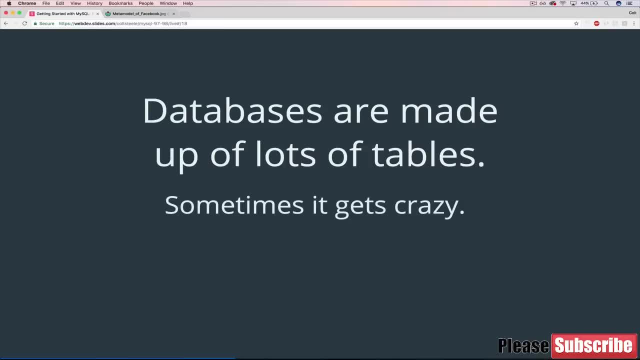 But for now we're not going to really worry too much about that, But just to show you, sometimes it does get crazy. You can click this link or I'll click it. follow my own instructions to see the breakdown of some of the tables. that Facebook's database or a social network. 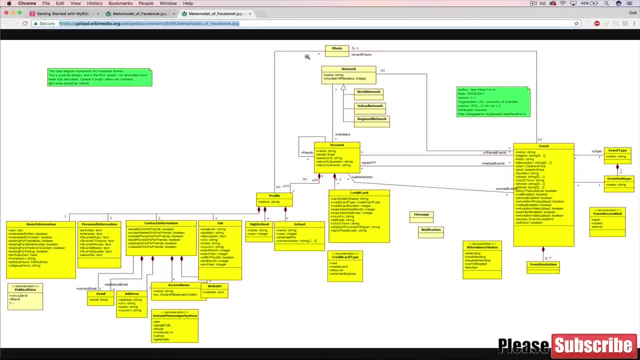 might use in their database. So this is not actual. you know this is not 100% accurate. There are things that are missing or incomplete, but this just shows all the different tables, or at least some of the different tables involved in a pretty complex app. So, as you can see, there's a bunch of them here. Things like 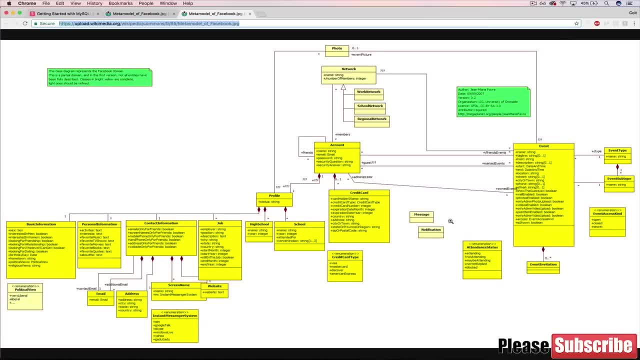 accounts and events and message and notification website screen name address, blah, blah, blah- All these different things to take into consideration. So things can get messy And as we progress in this course, you will start working with multiple tables. You'll see how. 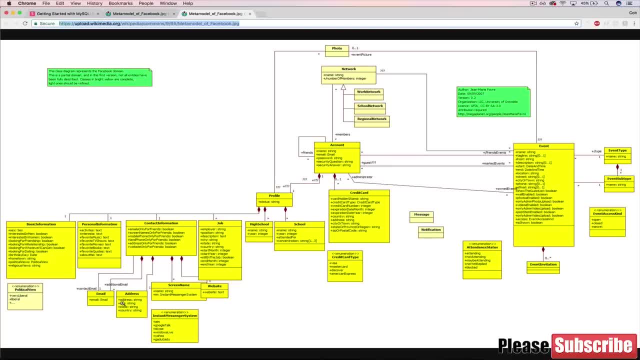 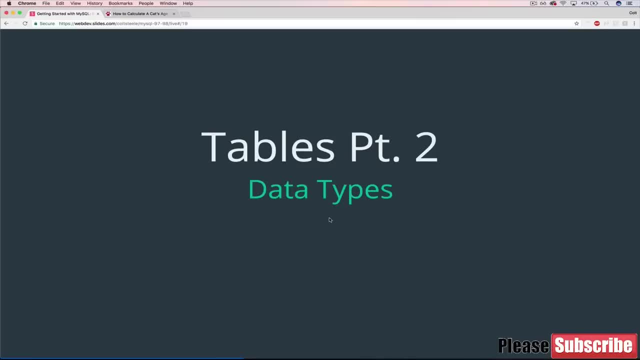 they connect, But we haven't even seen how to create a single table yet, So we're going to focus just on individual tables and then we'll move on from there. So the next thing we need to discuss around tables are data types. So data types are really, really important And to show 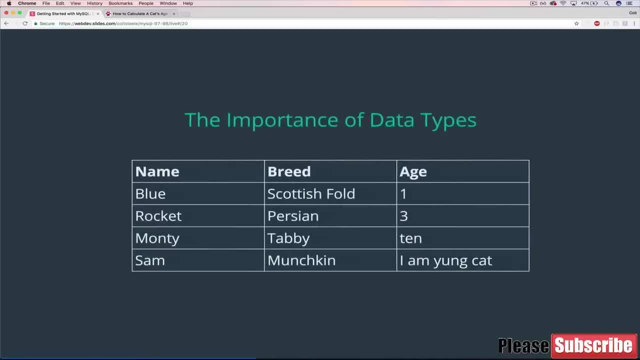 you what I mean, and first of all, what I'm talking about, when I say data types. let's return back to our cats table. So we have these three headers, three columns: name, breed and age- And here's an example. I changed some of the data just a little bit, So the names are the same. 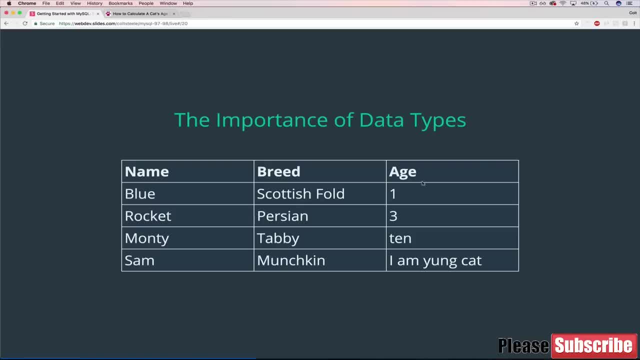 The breeds are the same, But if you look over at age, Blue is one year old, Rocket is three, But Monty now is 10.. The word 10. And Sam is crazy. Sam's age is. I am young cat, So what I'm trying to. 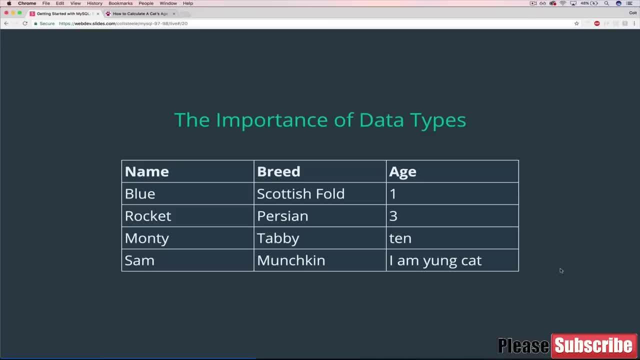 illustrate here is that we have inconsistent data. This is all text in text, But here we've got text with text And that is not good And it's actually not allowed in SQL at all. When you create a new table, you actually have to specify: name has to be text, Breed, has to be text Age. 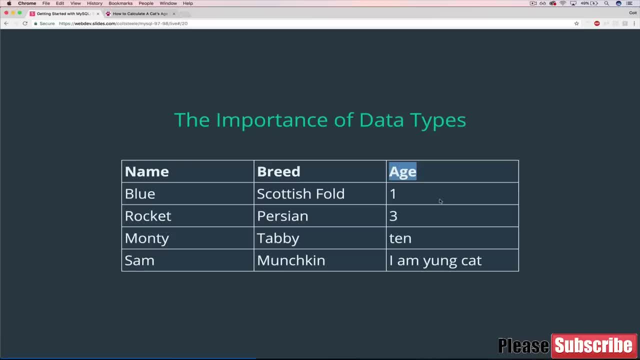 has to be a number And there are a whole bunch of different data types. It's not just text and number. In fact, those aren't even data types. Those are just what I'm calling them- the English version, But you'll see them in just a second. But to illustrate why it's so important that your data 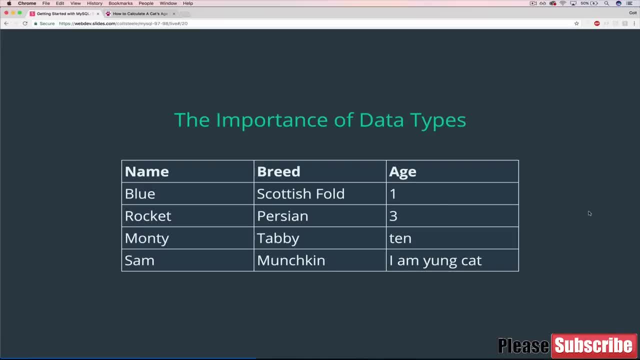 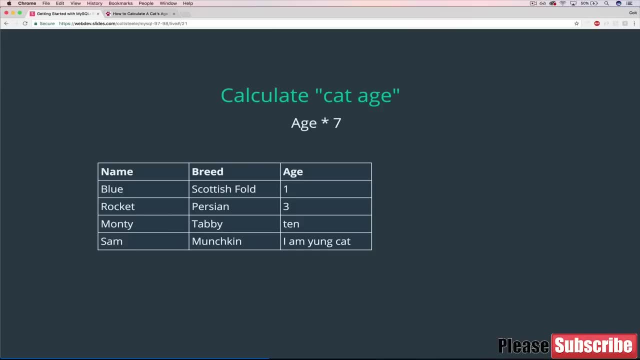 matches, That you don't have this inconsistent data And why SQL forces you to do this. Here's a little example. So let's say that you have this data in your database in a cat's table where, hypothetically, in a fictional world, you can have data that isn't all matching. So we have this numeric data mixed. 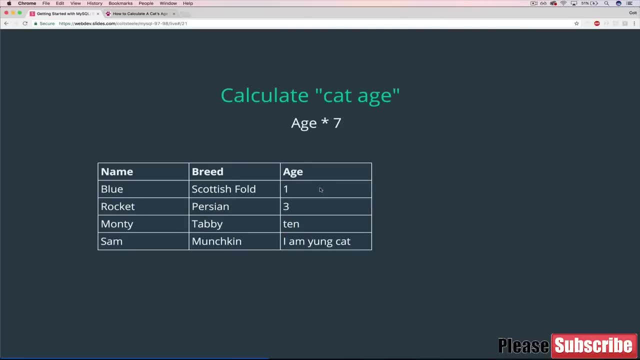 with text under age. So let's say, I wanted to make a really, really simple app that would take each cat's age in the database And then print out the converted or equivalent cat age, So from human years to cat years basically, which is sort of interesting. actually, in making these slides, I learned quite a bit. 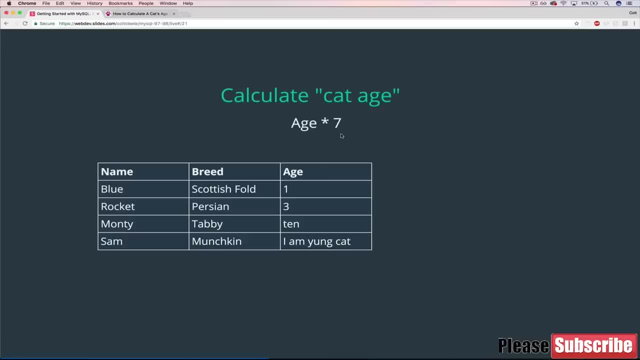 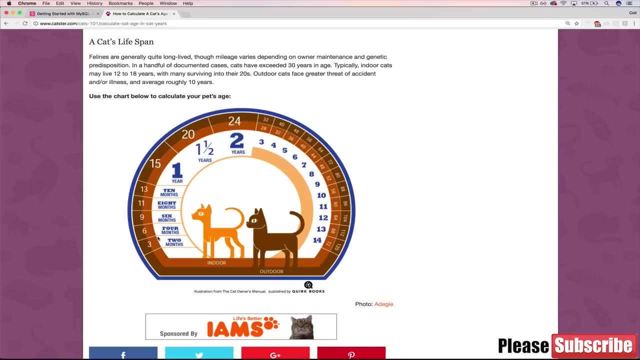 about how you calculate cat age, because for dogs there's this colloquialism: you can just multiply it by seven. For cats it's a little more complex. Apparently it's not linear. So if you look at this scale, when a cat is two months old it's three years. 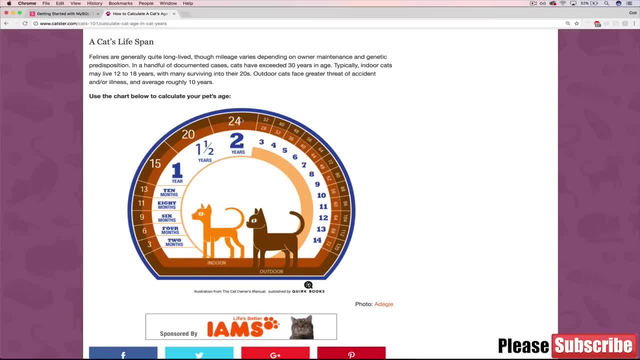 In human years. but then, as they get to two years old, it's suddenly 24.. And when they're 14, it's 72. So it's not consistent. So I just decided, you know what, let's just go with multiplying by seven it. 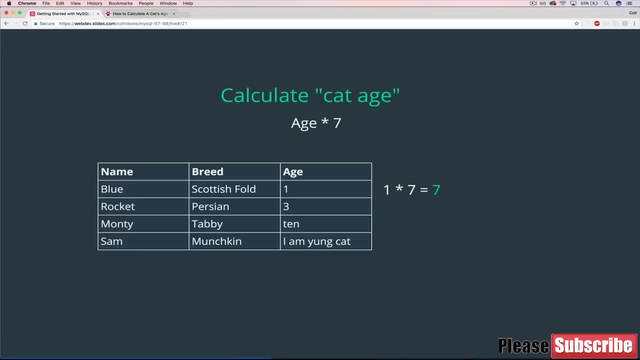 really doesn't matter. So our app takes the age of blue, multiplies by seven, no problem. Our app takes three, multiplies that by seven, no problem. But it has no idea what to do here. It, our code, doesn't expect text And it can't do that. the math And same thing with. I am young cat. 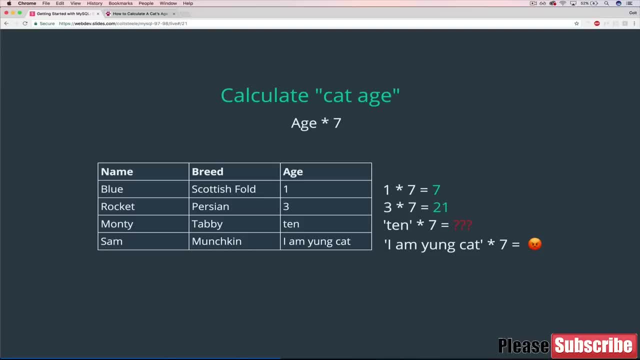 Time seven. it doesn't even know what to do, it just freaks out. So really trivial, stupid example, I know, But the idea here is important- that we have to have these data types established and that my SQL will enforce them. So when we create tables, we have to say exactly what data type we're looking for, Because this 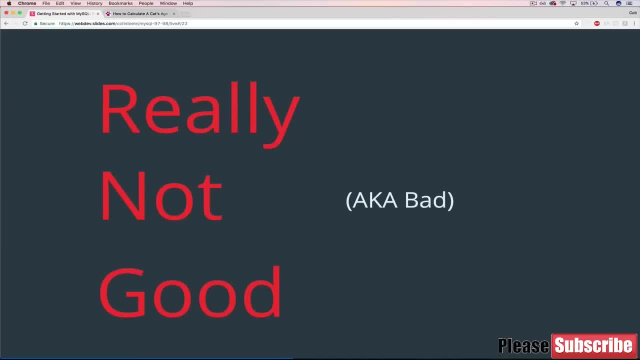 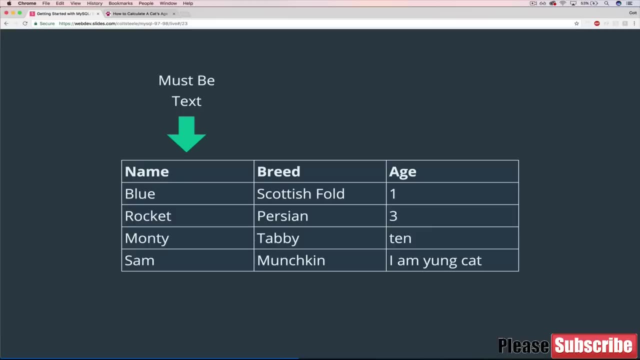 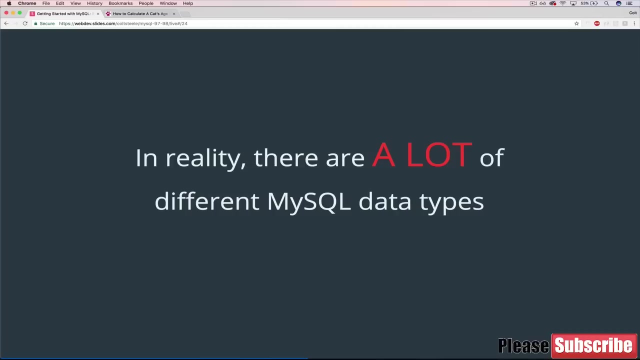 type of situation is really really not good, also known as bad. So, returning to our cats table, when we're creating it we'll have to say: must be text, breed must be text, age must be a number. So in reality there are a lot of different MySQL data. 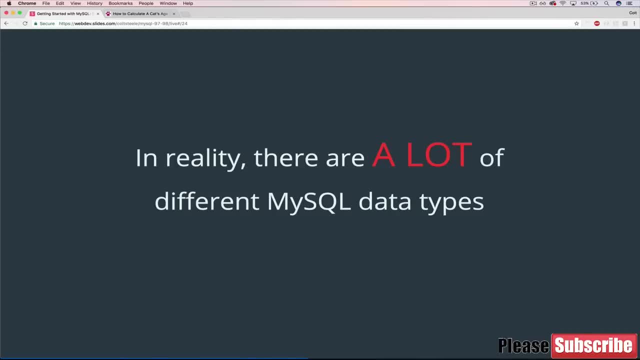 types it. like I said, text and number are not real data types. In fact there are a ton- in my opinion too many- and it gets pretty confusing, especially when you're just starting out. it can be intimidating. Just to 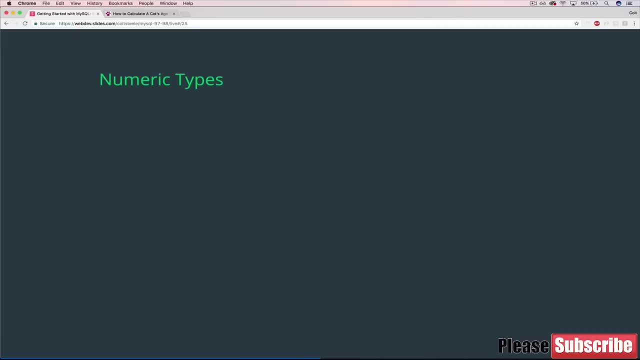 show you exactly what I'm talking about. I put together a list of all the different data types, So all the numeric types, basically the different ways of representing numbers. we've got ints, small ints, tiny ints, medium int, big int. 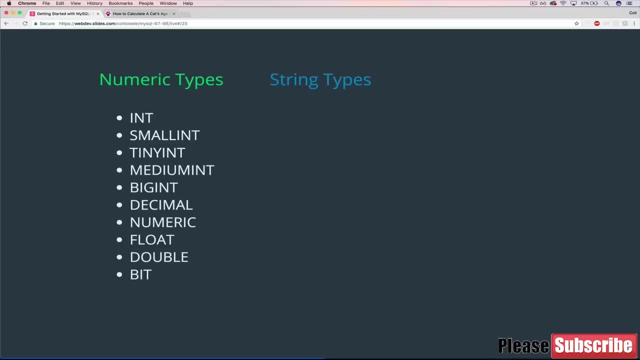 decimal numeric float, double bit then under string types. so these are ways of representing text, basically: char var. char. binary var. binary blob. tiny blob, medium blob long. blob text: tiny text, medium text long. 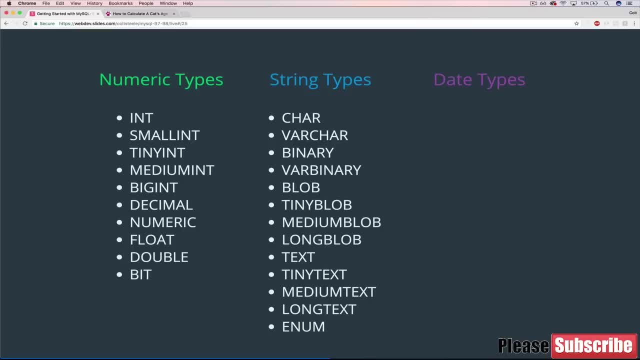 text and then enum, And then finally, we've got date types, We've got different ways of representing dates, We've got date, date, time, time stamp, time and year. So yeah, it's kind of crazy, I know. 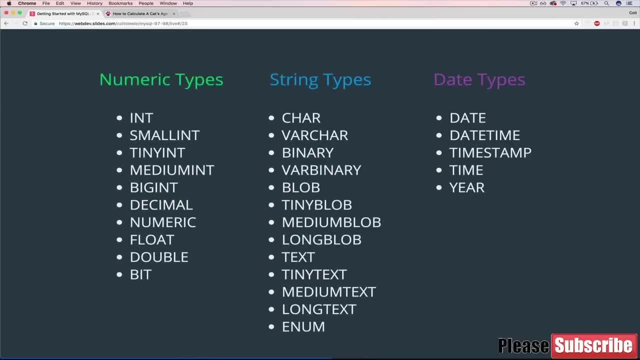 Fortunately, you don't have to know all of those at any given time- absolutely not. I had to spend a decent amount of time, even digging through the documentation, just to find all of these, because the reality is you don't use them most of the time, or you don't use all of them. 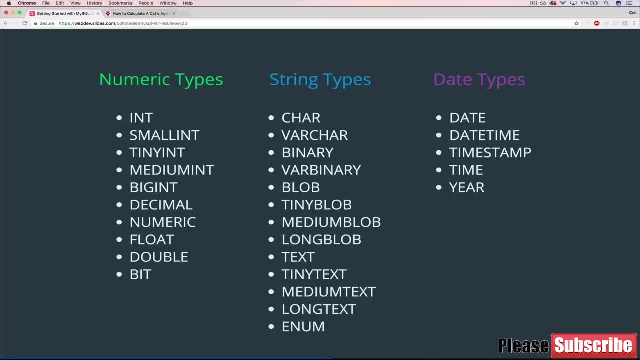 You figure out which ones you need depending on a given situation. you use a subset, normally, that you're comfortable with, and then eventually you may have to switch things out and change from using a medium int to a big int or or actually, more realistically, an int to a big int or something like that. 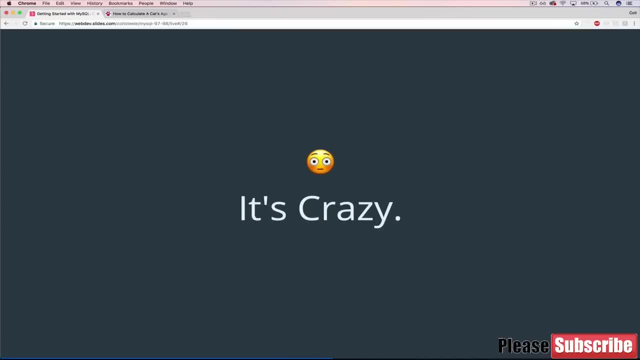 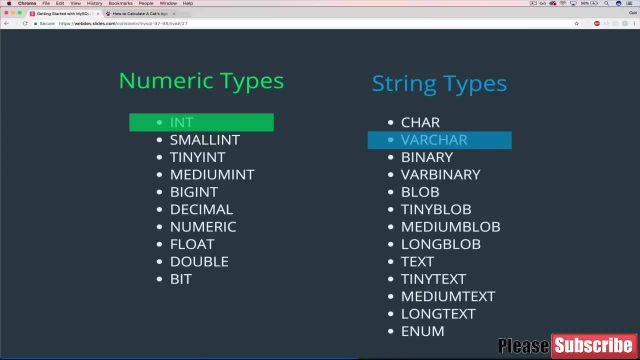 But we'll get there For now. we're gonna accept that it's crazy and we're just going to whittle it down and focus on two. The first one is int, for our numeric type, and then var, char, for our string type. 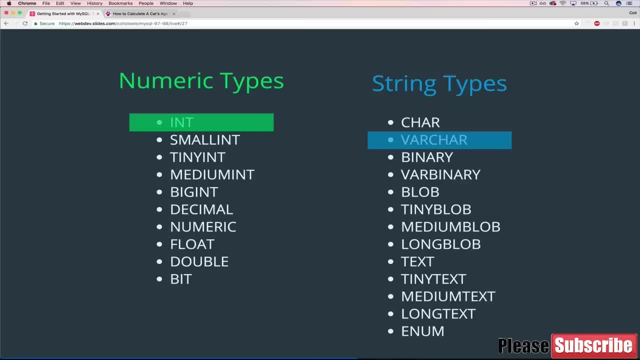 So to represent numbers, we're working with int, and then to represent numbers, we're working with var, char. so to represent numbers, we're working with int, And then to represent numbers, we're working with int. and then to represent numbers, we're working with equals, and then to represent 2.. 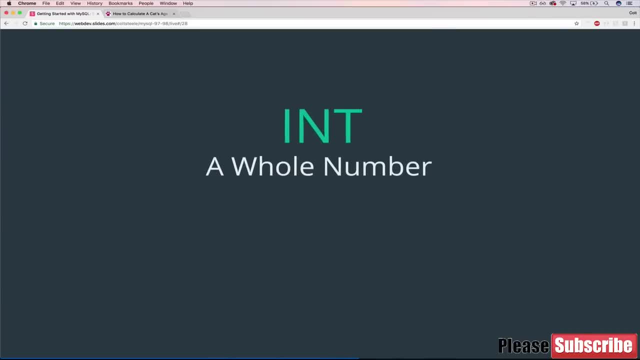 text and strings. we'll work with varchar. so we'll start off with int. so int represents a whole number, so we can't use it for decimals, and it ranges up to this gigantic number here. basically, it's big. however, if you need to store numbers larger than that, that's when you can start. 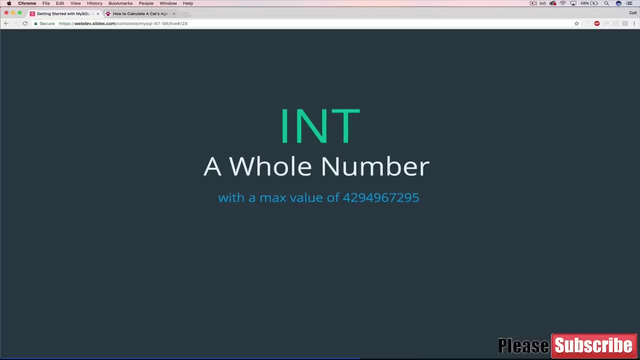 looking into some of these other data types but like big int. but we're not going to worry about that because for now we're storing things like cat age. so this is an int. here's another int. it can be negative or zero, or big or 42, so that's pretty much it to ints. then varchar is a way of. 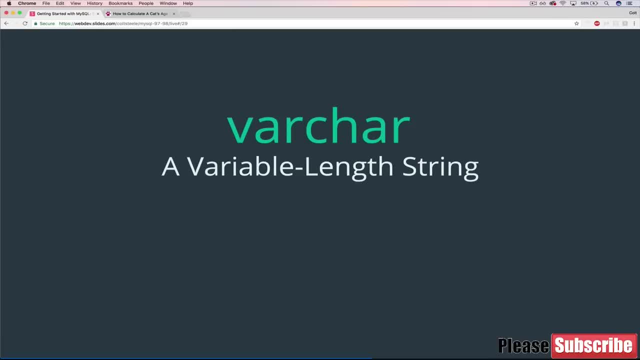 representing text or strings and its variable length. so you may have noticed that there was char on there and varchar. well, char is a fixed length, so that means that you can store things like cat age and it's variable length. so you may have noticed that everything in that column has to be the same length. It has to be 10 characters or something. 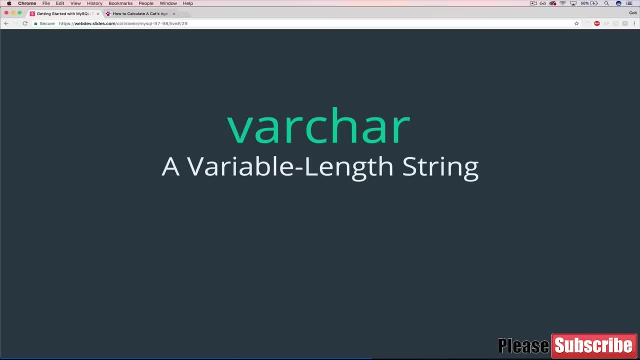 But Varchar allows us to have a variation in that, which is what we want most of the time, And it's between 1 and 255 characters, So things like coffee, or negative 9,999, the string in quotes, So it's not a number Or this, whatever this is, Or capital L Or a sentence, as long as 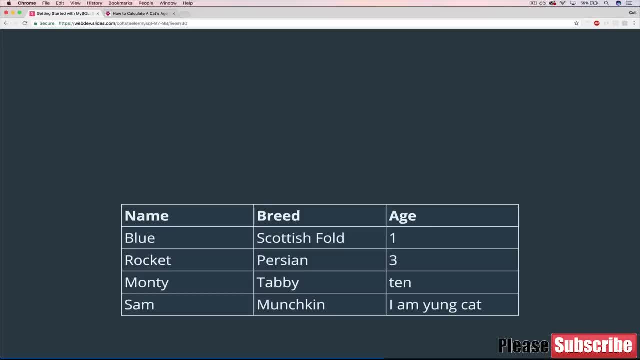 it's fewer than 255 characters. So, returning to our cats table, we would say that name, which must be text, would be Varchar, And notice that I have these parentheses here and a number inside. So when you use Varchar you have to specify a maximum length, So in my case I chose 100.. I could go up. 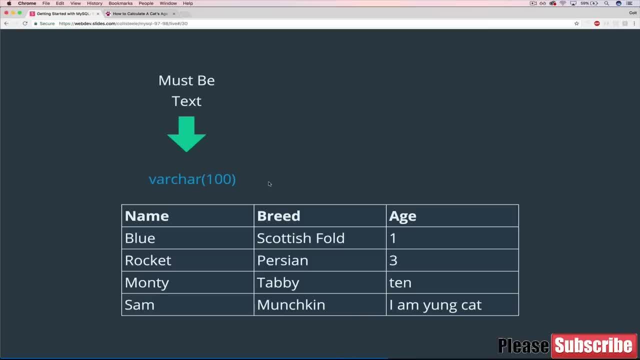 to 255. But I just don't want to have any giant names. But that's all that it does here. So it specifies where the cutoff point is And if I go beyond 100 characters, if I write 300, or 200 characters, all that will be stored is from the first character to the 100th character. 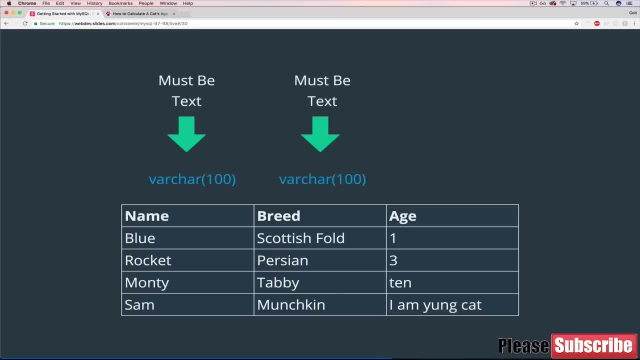 So breed. I did the same thing. It's Varchar And I did 100 again. But that could change If we wanted them. if we wanted to restrict breeds to be shorter, we could change it to be 50 characters And then for age, which must be a number we just use int We're just working with. 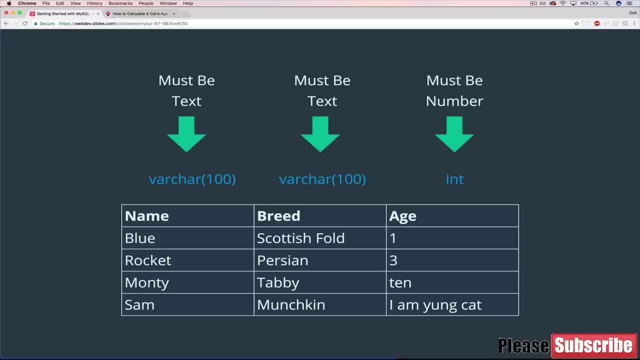 whole numbers We're not going to worry about. my cat is 1.2 years old or anything like that. Okay, so that's all we're going to do for now with data types, Basically high level overview, And we saw two of them in particular: Varchar and int. Next up, we have a really quick activity. So 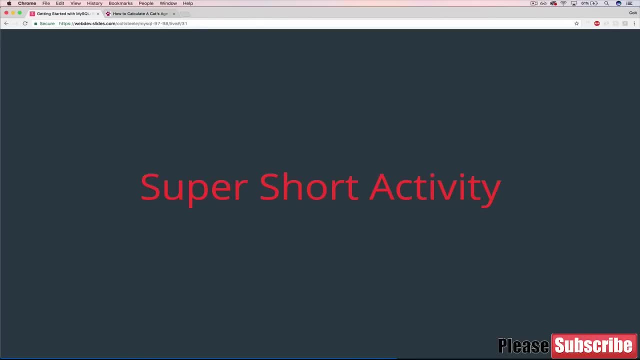 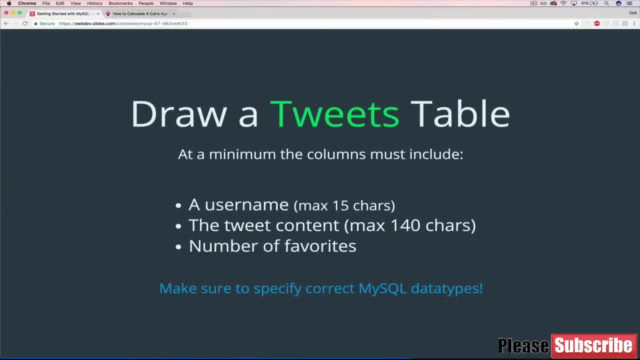 as I mentioned, we have a really quick activity now, And the point here is to get you thinking about data types and thinking in data types or in terms of data types. So what I'd like you to do is draw or write or just think about a tweets table, So modeling tweets, If you're not familiar. 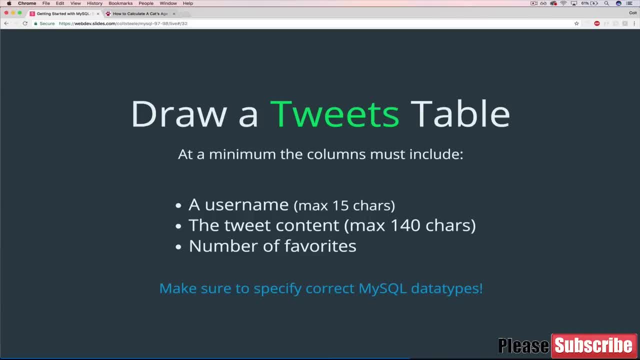 with Twitter. that's going to be a tough one. So I'm going to go ahead and do that, And I'm going to go ahead and do that one, I guess. But basically there are three things I need you to at least. 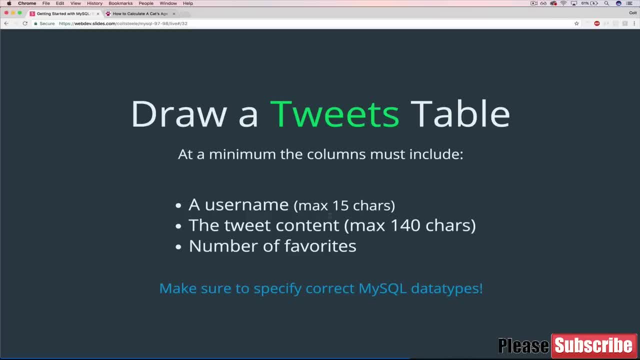 three things that I want you to model, And these are the columns. So a username. So when someone tweets, let's say I tweet and I have- I don't actually use Twitter, but if I had an account and I called it coffee lover cult, I mean that's just terrible. But if I did, it would need to be. 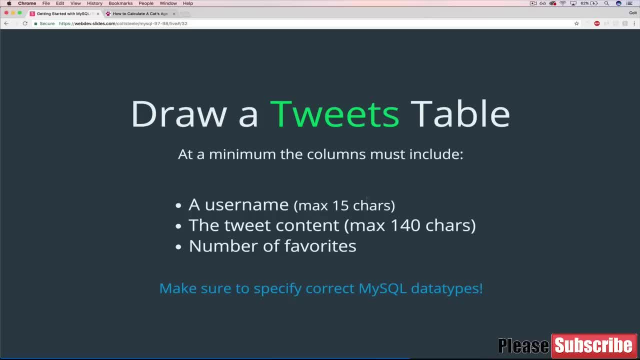 maximum 15 characters long. So how do you specify that? What data type is it? Then? the content of the tweet, So whatever the tweet is itself can't be more than 140 characters. And then the number of people that have favorited that tweet, basically liked it or hearted it. So you don't have to draw. 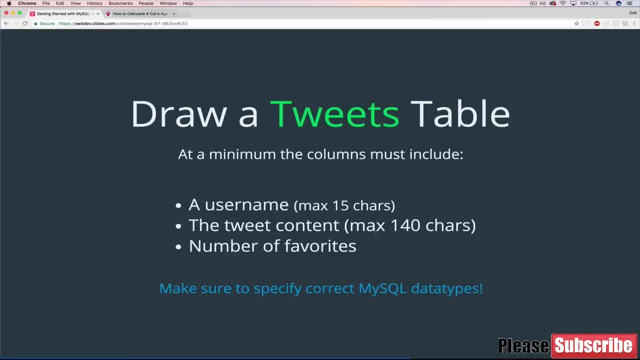 it out. But if you want to draw it out in that tabular format and then fill in some fake data or even real tweet data that you find, go ahead and do that. But just think about what these data types are in terms of what we just learned, And there's really only two choices that we saw, So hopefully, 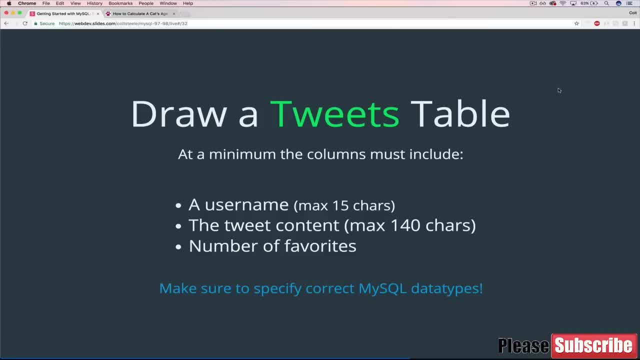 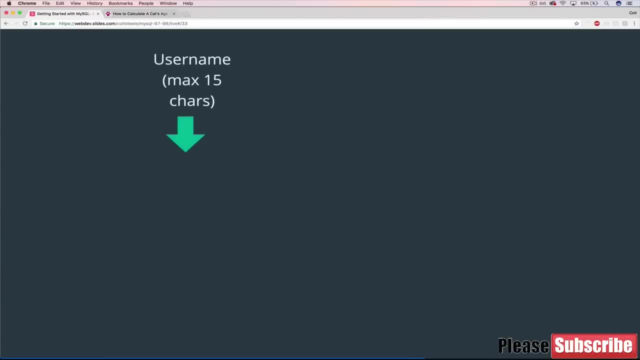 it's not too difficult, So we'll be right back with a solution. Okay, So let's start talking about the answer. So we had username which was a maximum of 15 characters. That would be a VAR char And you would put 15. 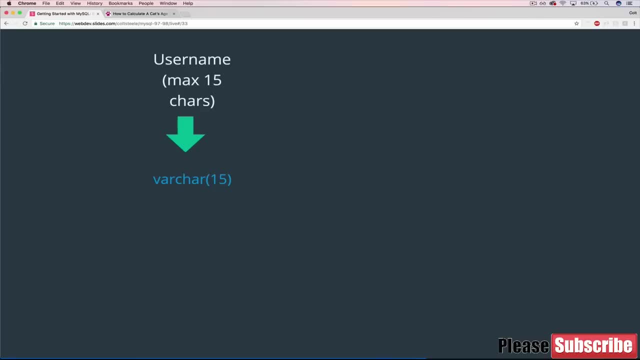 in the parentheses to specify that it's no more than 15 characters. Then we have content of the tweet, max of 140.. It's very similar. It's also VAR char- it's text, But this time we restrict it at 140 characters. Then we have favorites, which is just a number, So we use int And then 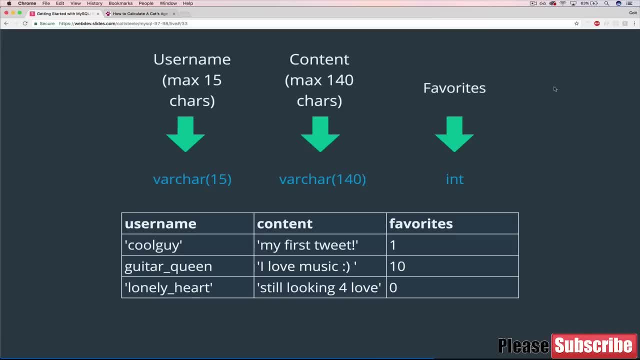 here's some mock data that I added, If you want to take a look. we have cool guy who tweeted my first tweet And I was one person who liked it or favorited it. Then we have guitar queen who tweeted: I love music, smiley face, how endearing, And we have 10 favorites on that. And then lonely heart. 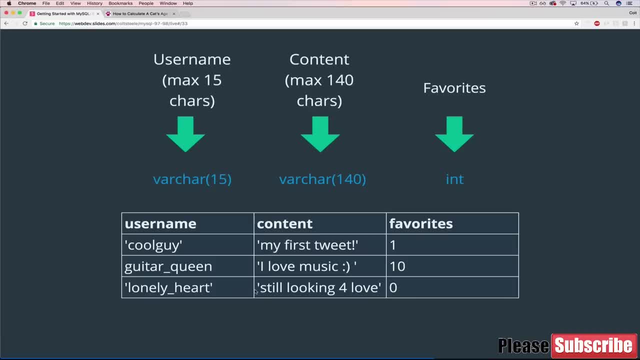 this sad guy or gal Who tweeted still looking for love And that has zero favorites because nobody wants to be depressed, All right. So next up we're going to see how to take these data types and actually tell SQL or MySQL how to implement a table using those data types. So now that we've learned how, 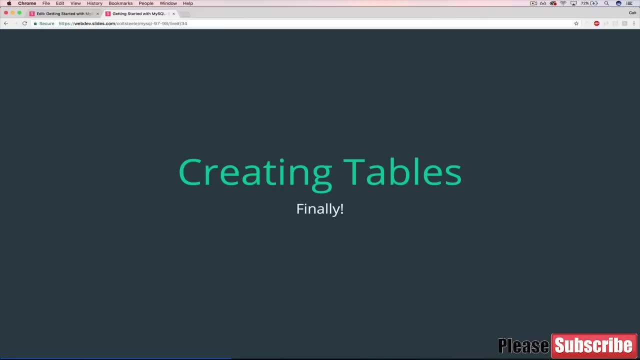 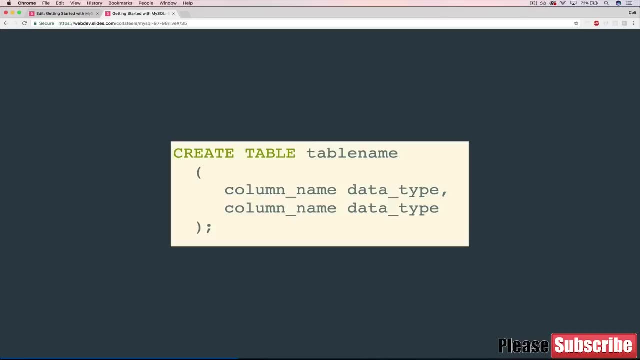 tables work and we've seen a little bit about data types. we finally get to start creating tables. So here is the magic syntax for creating a new table in MySQL. Here is the generic version, So it's create table and then the name of the table, So cats or users or people or. 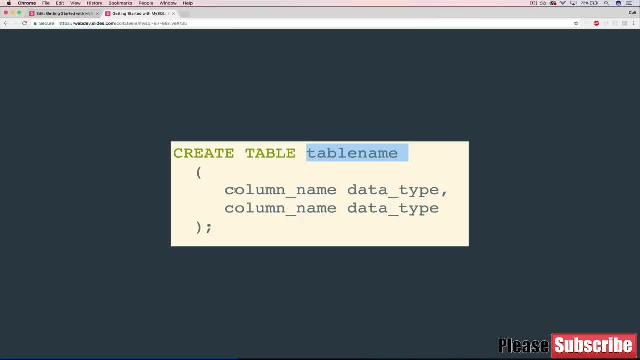 results or whatever it is, and then in parentheses a column name and then a space and the data type. And there are a few other things that can come along with the data type, But for now we're just talking about data type. So a column name, like age, is an int, Or address is a varchar or varchar. 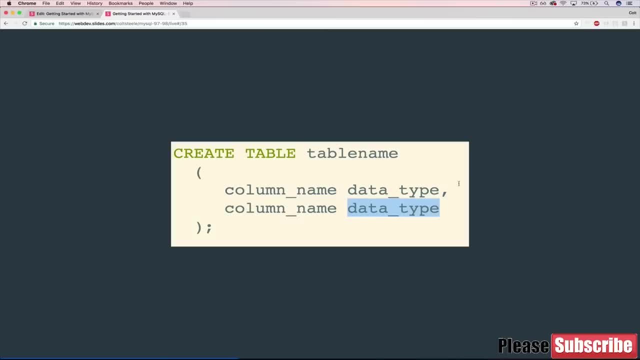 However you want to pronounce it. So that's the main idea. And you keep listing these columns, as many as you need. it could just be one, it could be 20.. And you separate them by columns, excuse me, by commas, And then, when you finish, you add your semicolon, And that's that. You don't have to. 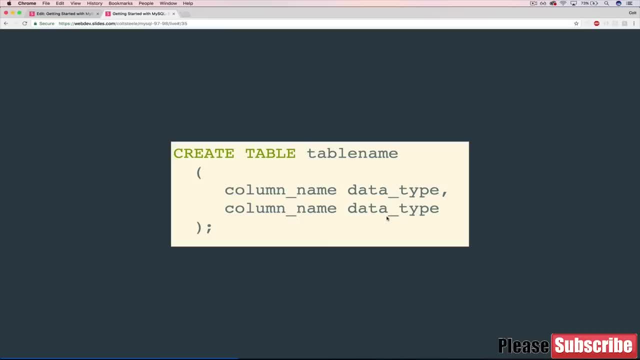 format it this way, on separate lines, But I think it's easiest to understand. It's definitely easier to read when you get much more complex ones, But you could do it all in a single line, just like anything else in MySQL. So here's an actual example using our cats table. So we're just working with name and age create. 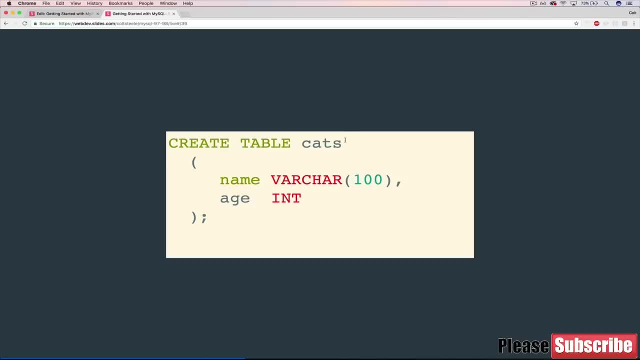 table cats. One thing I should point out is that table names should be pluralized. So it doesn't actually matter for the mechanics or behind the scenes, it won't change anything. But you want to just follow this convention, use plural, because that's what a table describes- is multiple cats. 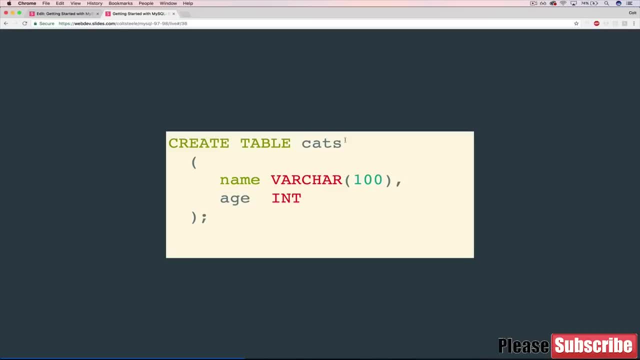 or people instead of person, or payments instead of payment, and so on. Okay, so we have parentheses and then we list our columns and their corresponding data types. So name will be a varchar with a 100 character limit, comma. age will be an integer. So let's hop over to. 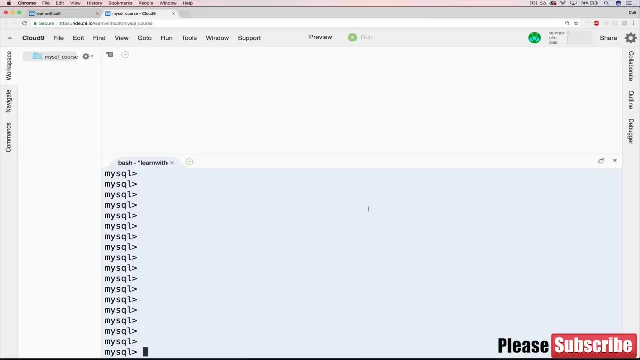 cloud nine and see if it works. So the first thing I'll do is just make a new database. You don't have to do this if you're following along, but I'll just call one cat app- Oops, forgot my name. Then we will use. Okay. so now the next thing we'll do is create table cats And then we can. 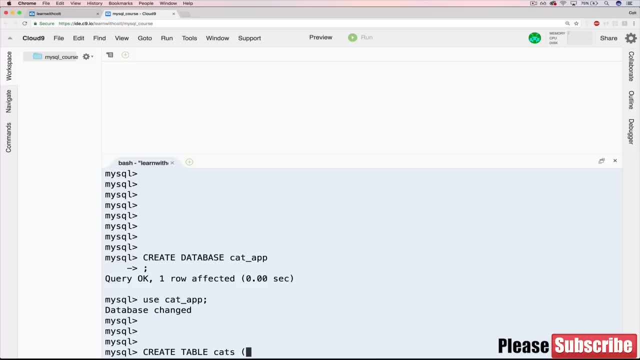 either do parentheses here, And that's what I usually do when I'm working in the MySQL command line or in the shell, So you don't have to worry about spaces too much. So create table cats, And then we'll say: name is a varchar. 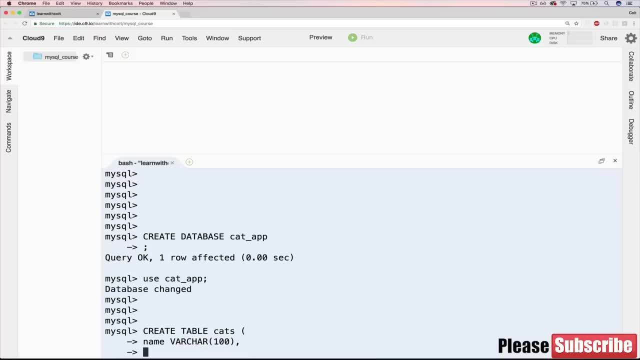 100, comma. age is an int, And then we'll close our parentheses with a semicolon Query. okay, zero rows affected. Perfect, It appears to have worked, Or at least we have to trust that it worked, Because right now we don't have a way of testing that, But we will in the next video. 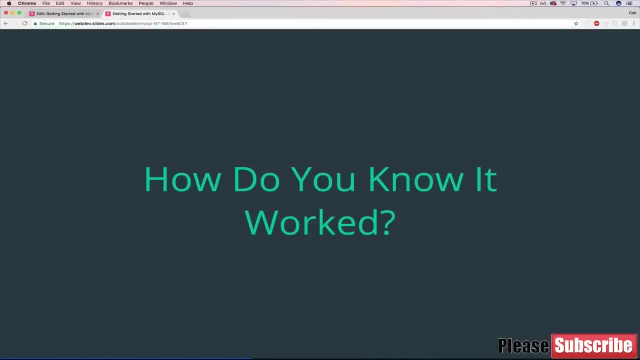 Cliffhanger. So we left off by creating a new cats table And it said: query: okay, But the question is: how do we know that it worked? How do we know that it worked? And then we'll 今回 m? ys, We will challenge our cat app to show that it did what we wanted it to do. So there's. 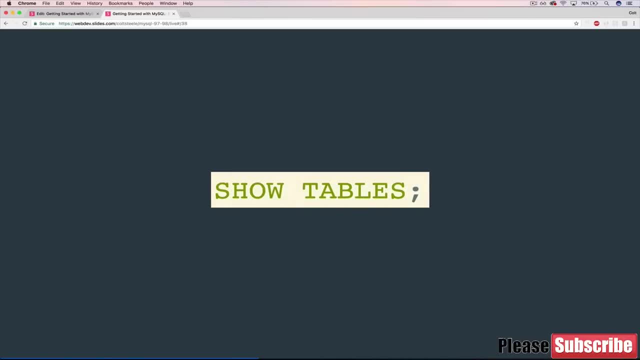 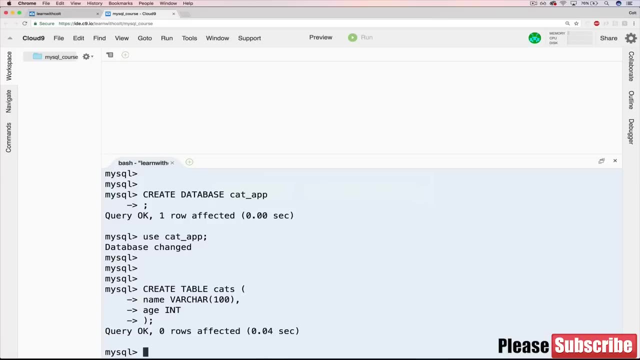 a couple of options. The first command I'll show you is pretty straightforward: Show tables. Very similar to show databases. It just is going to show you the current tables in your database. So we can try that now, And c vaude nine will do show tables just like that, And it tells us tables in cat app. There's. 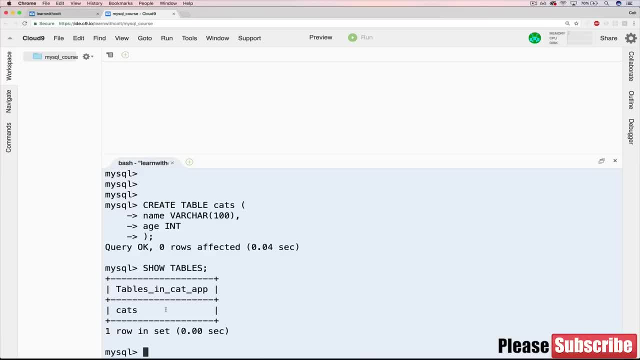 one called CATTS cats. so that's great. it tells us that there is a cat's table, but that's pretty much. it doesn't say anything about the contents of that table. what are the different columns in it? which brings us to our next command, which is again using 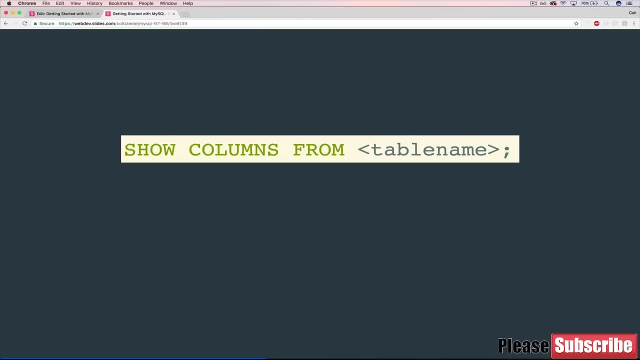 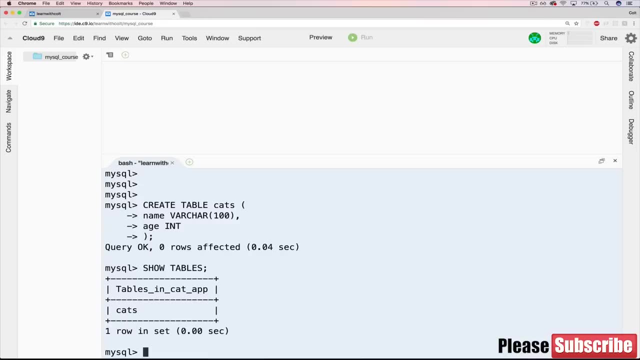 show, show columns from a table name, so in this case we would say show columns from cats. so let's try it out now and, as you can see, we get some nice little table back here that says we've got two fields: name and age. name is a varchar. 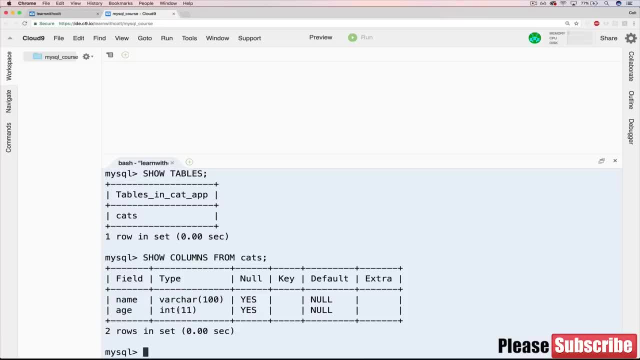 with 100 limit and age is an integer, and don't worry about this 11 for now. then we've got some other data that we're also not going to worry about, because we're going to talk quite a bit about it in the next section, but you, there's. 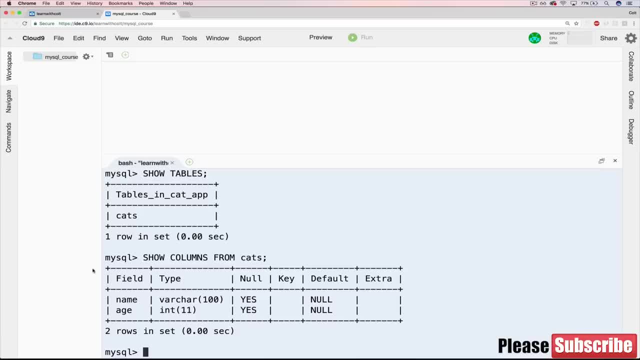 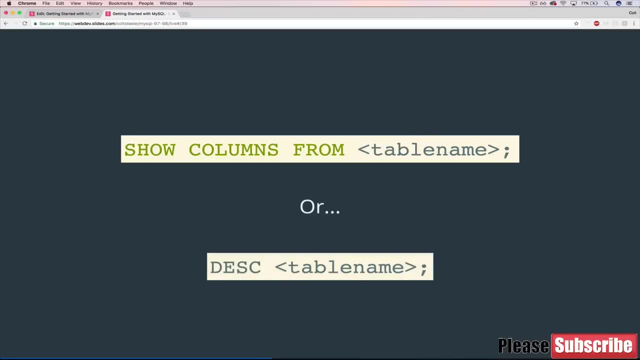 some other categories here that we're just going to ignore, but this is what we want. name: varchar, age, int, perfect. one other thing I'll show you is that you can use a shorter version. technically these are slightly, slightly different commands, but used in this context there is no difference, so we can use describe. 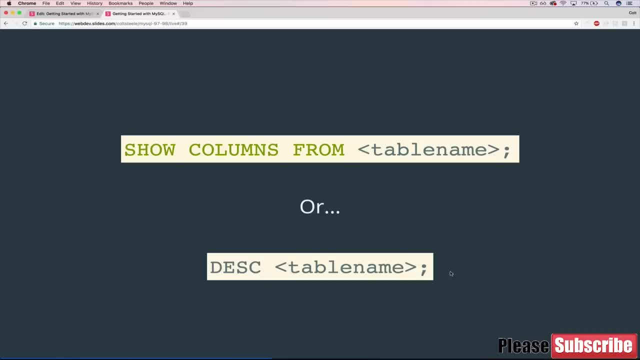 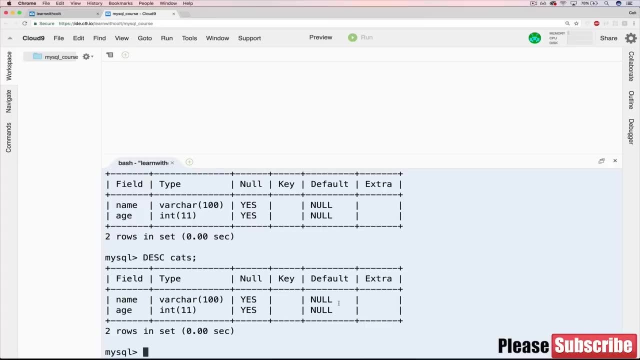 or DESC, a table name, and that's my preference. it's shorter, easier to remember, so let's try that out. describe cats: you can see we get the exact same printout. so I did say that you could use them differently in a more advanced setting where you can basically pass in some. 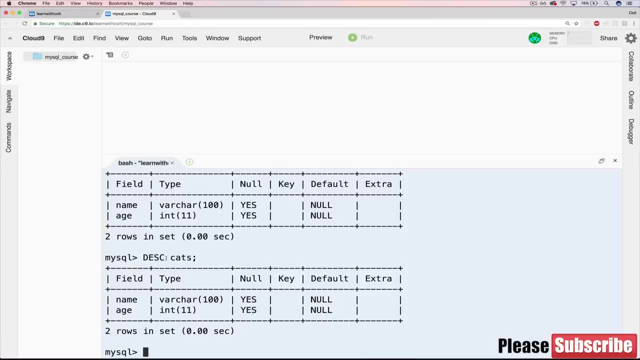 other things to describe. so, anyways, it doesn't really matter, but I just want you to know they're not exactly identical. it's not like one is a shortcut for the other, but they do the same thing in this context. all right, so this video was pretty quick. it was just about kind of testing and making sure. 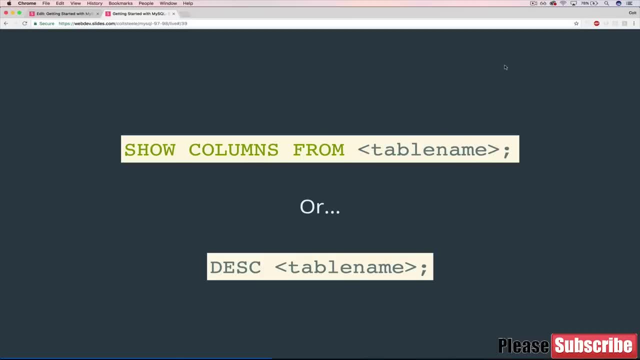 that when you create a table, it's created accurately and that you can one tell that the table is there using show tables but, more importantly, see the actual columns in that table using these two commands. okay, so the last little bit of syntax we'll learn in this section has 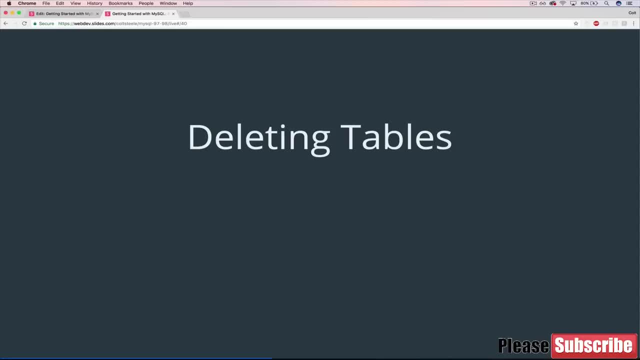 to do with deleting tables. we've seen how to create tables. we've seen how to describe or show their columns. we haven't seen how to put anything in those tables yet. that's coming up next, in the next section. but the last thing we'll do is see how WE delete them. so think to yourself for a moment and make 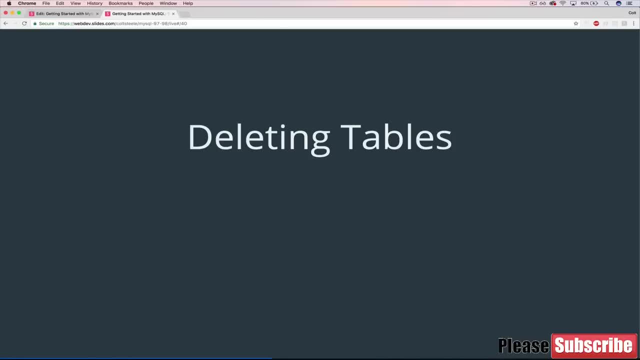 sure that you're going to get the two comments fuzzy and educated and we'll just skip those and you'll get the third one. I should, And that's what I always like for a table. so it's going to matches tools, not to mới moment. what's your guess about how you delete a table? My hint is that it's pretty similar to. 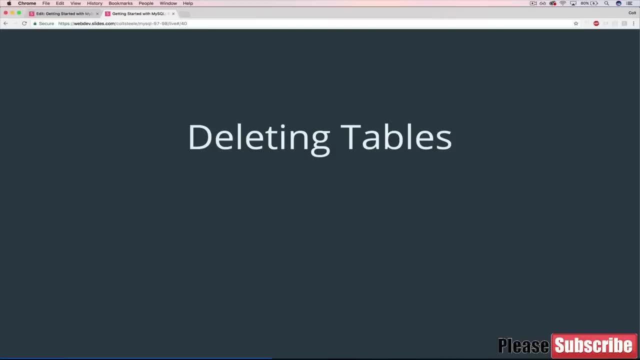 how. we've seen how to delete something else before in MySQL. Okay, so think about that and I'll just wait here for a second. I guess maybe make a coffee, All right, so the magic is drop table and then the table name. So rather than drop database, we're going to say drop table. 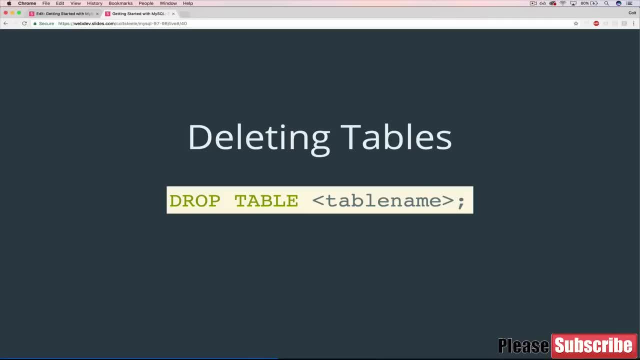 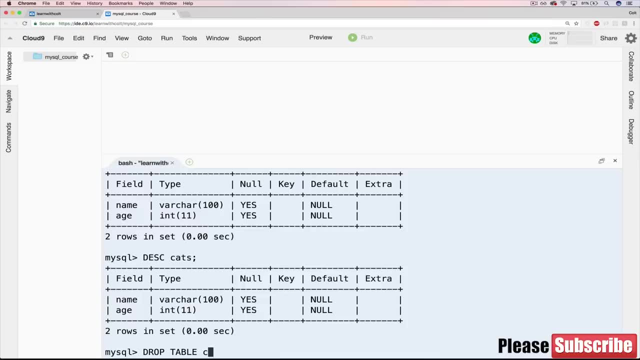 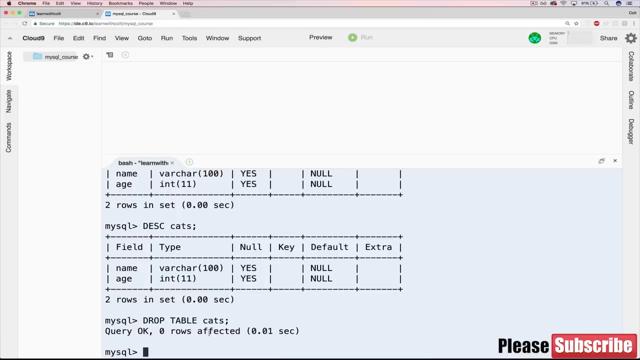 and then cats in our case. So just to prove to you that that works, let's give it a shot Back in Cloud9, I will type drop table cats and this is permanent. it's going to disappear, It tells us. query okay, To make sure that it's actually gone, we could use a couple of different. 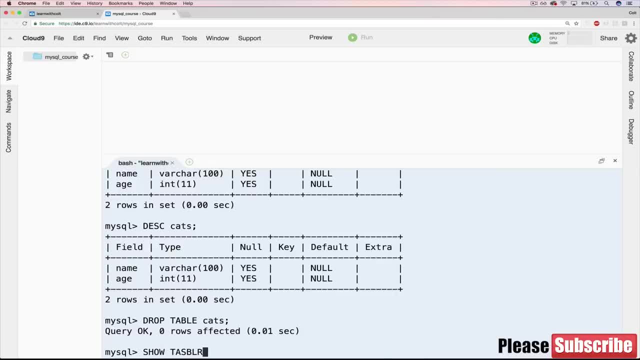 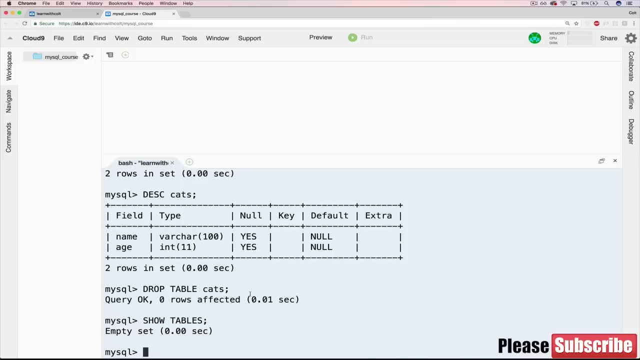 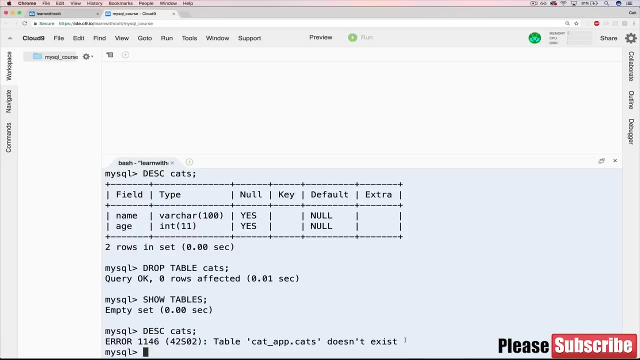 things it's up to you We can do: show tables and it tells us empty set, there are no tables here, whereas before, when we did that, we got data And if we try to describe cats now we get an error because cats no longer exists, so it can't even show us. 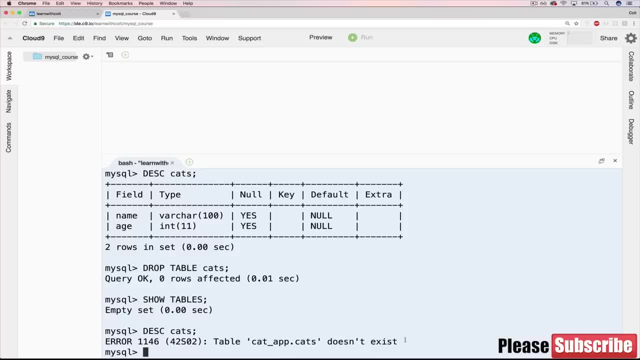 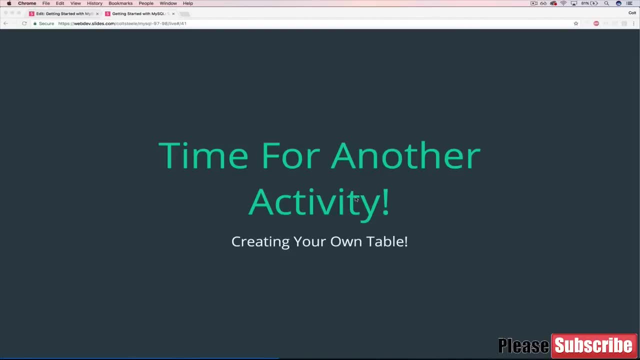 the columns because it doesn't exist. So that's all there is to dropping or deleting a table, very similar to dropping a database. So to close out this section, here we're going to get a little practice with data types and the syntax for creating and deleting tables. So one more activity. 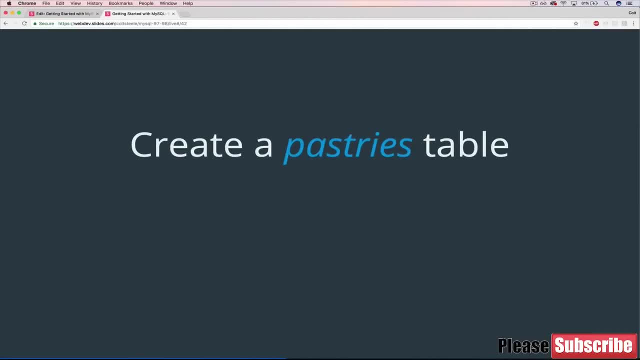 This time I'd like you to imagine that you work at a pastry shop. So you're going to manage- and I manage in air quotes that you can't see me doing right now, but you're going to manage a pastry shop in the inventory for these pastries. It's 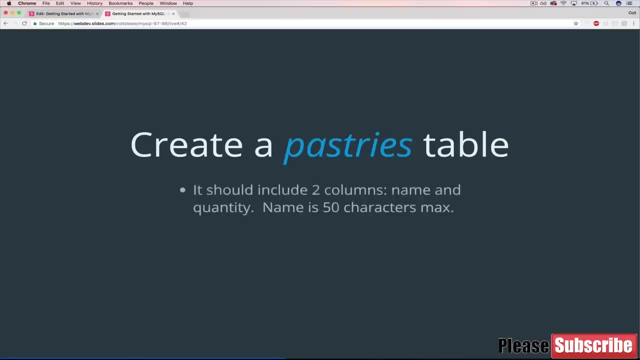 going to be very simplistic, but you'll need to create a pastries table and there should be at least two columns. If you want to add more, that's fine, but a name for the pastry. so what is it? a croissant, a chocolate donut, whatever it is, as well as a quantity. 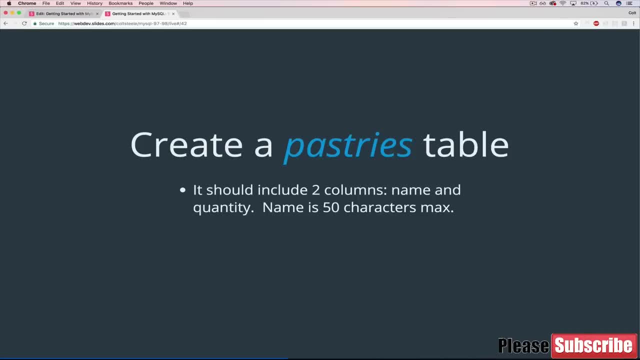 Which should be a number, So I could go in and see that there are ten croissants or five chocolate croissants and so on, But we won't fill it with data because we haven't seen how to do that. So 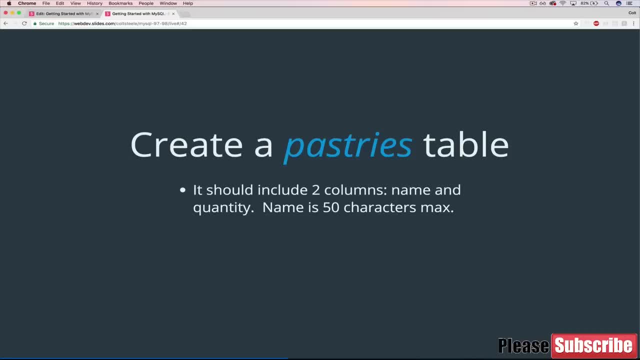 we're just defining the table and the columns, So I'd like you to do that. Then use a command to inspect your table and the columns using the MySQL command line interface. So one of those short little commands we saw just to make sure, basically to check your work And then, lastly, delete all. 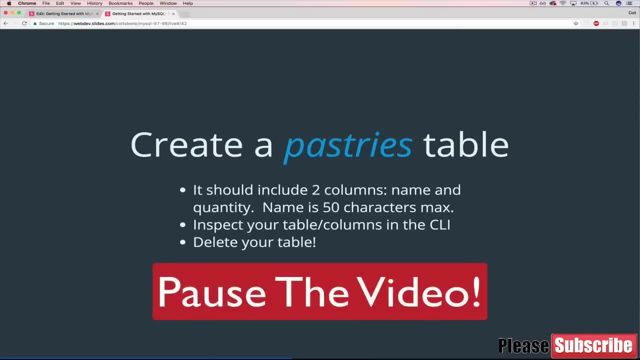 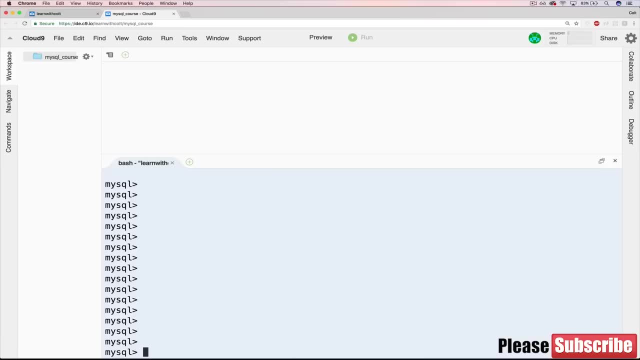 the tables. So pause the video if you'd like go through this and come back when you're done And I'll be here. Okay, so I'm back in Cloud9.. I'm actually still. if I select database, I'm still. 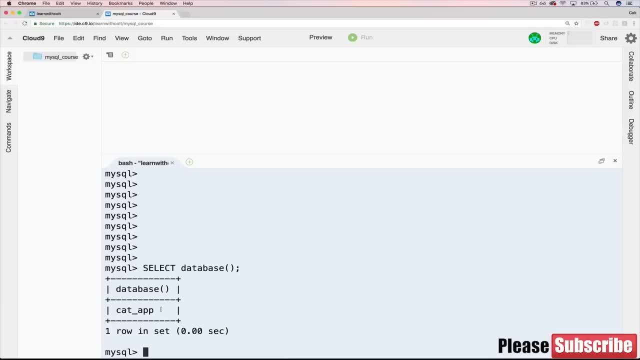 using CatApp. There are no tables in there right now because I deleted the cats table, But I'm just going to put our pastries table in here, even though it has nothing to do with CatApp. Maybe it's a cat bakery or something. I've seen dog bakeries, so 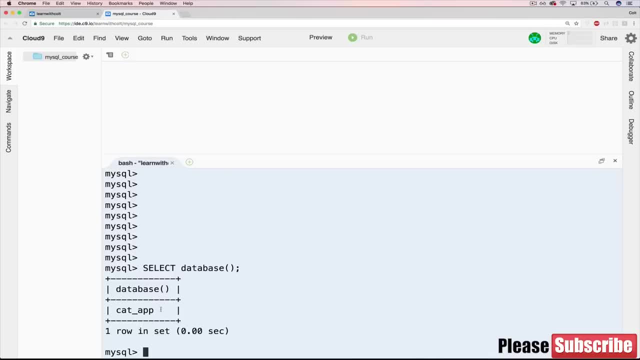 Maybe we're not too far off, But anyways, it's just a silly exercise. So we want to create a table, So create table, And then the name of the table will be pastries, plural. Then in parentheses- And I'm going to do it on one line, just to show you that it's not a problem- So we'll have the: 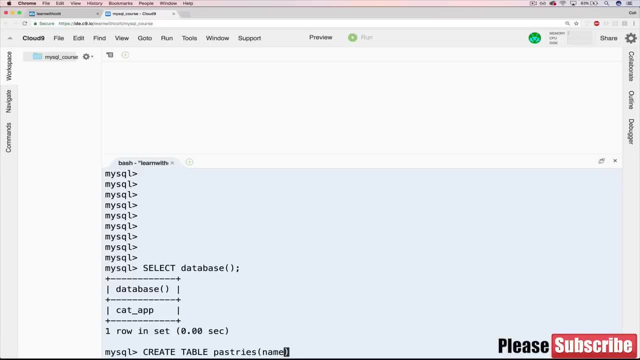 name of the pastry. And one thing that you may be tempted to do if you come from some other databases is to put a colon there. That's something I find myself doing just from experience that I have with some other tools, But you don't want that there. So if you see me doing that, hopefully I catch myself. 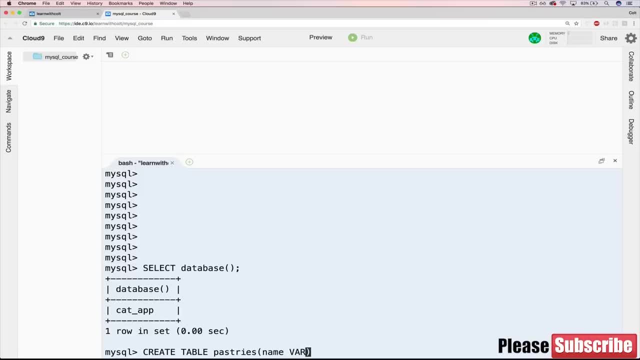 Create table pastries. Name is going to be a varchar And it should be 50 characters maximum, So in parentheses, 50. And then we have age. Excuse me, We have quantity. If you wanted to abbreviate that with just QTY, which is what you'll see, pretty. 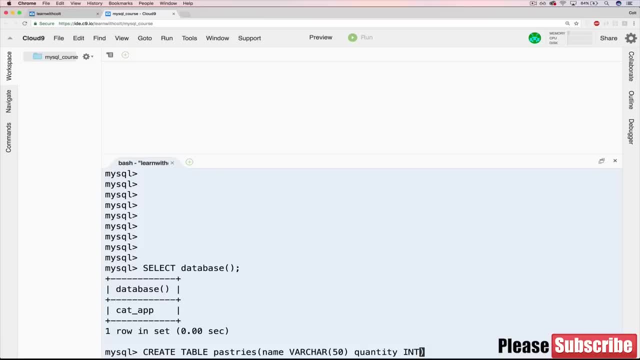 commonly. You could do that as well, And that's just an integer. Then we need our semicolon to end it. We hit enter And we have a nice little error message. So that was accidental. I'm not going to try and play it off, like I did it on purpose, But I am going to leave it in here And that's mainly. 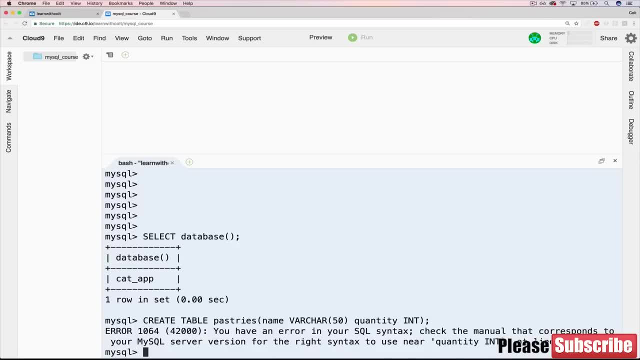 because it's something that pops up pretty commonly. People aren't perfect. At least I'm not, especially when I'm recording. I've got a lot of stuff to worry about. Can you identify what went wrong? I'll give you a hint. I'm just missing one character: Yep. If you got it, I'm missing a comma here. 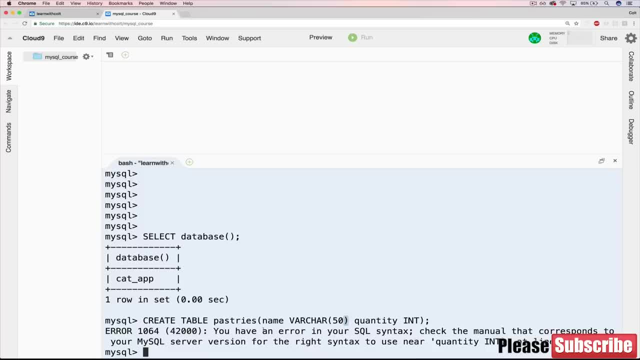 And the error messages aren't always that useful. But it tells me there's an error in my syntax And it's something near quantity int. So right before that I'm missing a comma And it's treating all of this as name, which is wrong. We need that comma there So we can recall the line. Go back. 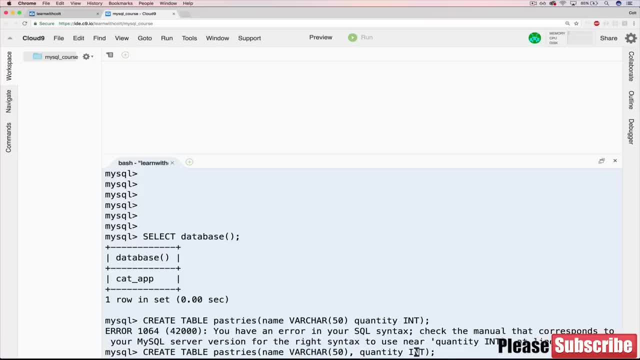 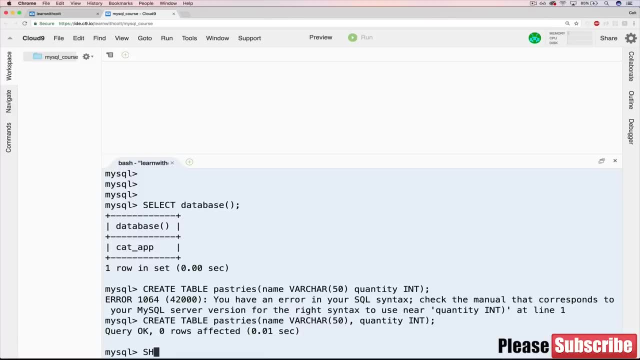 And insert our comma. Now, when we do it, we get query OK And we'll move on to the next part, which was to make sure things worked. So we could either do show tables And then we can do show. Let's do. 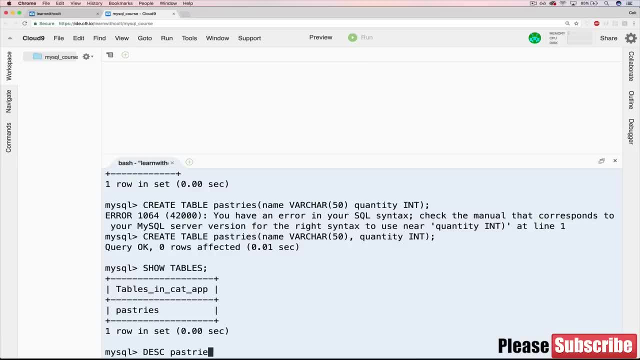 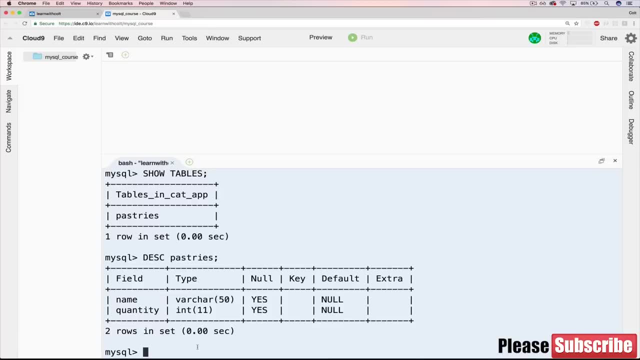 describe, Describe pastries. Perfect Name: varchar. quantity is an int. And the last thing was to drop our pastries table. Drop Table Pastries, Goodbye pastries. And just to verify it worked, let's do show tables again. And 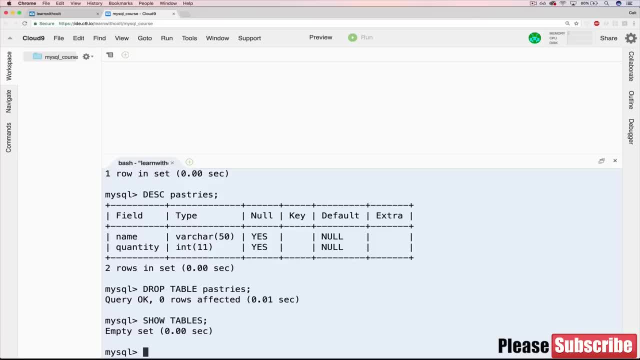 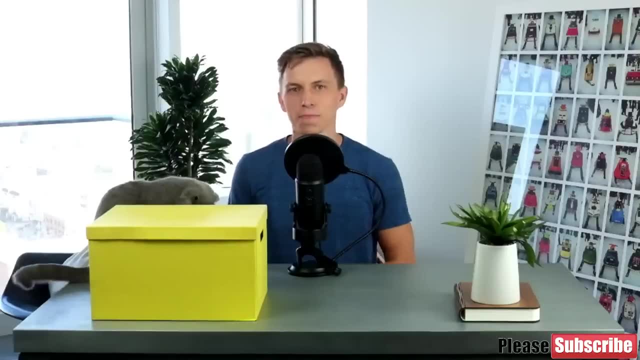 there's nothing here, Perfect. So the next section is all going to be about inserting data. We make tables. They're empty. How do we get stuff in there? Hey, welcome to the next section. So let's recap what we just saw. in the last section, We basically saw how to make databases and then how. 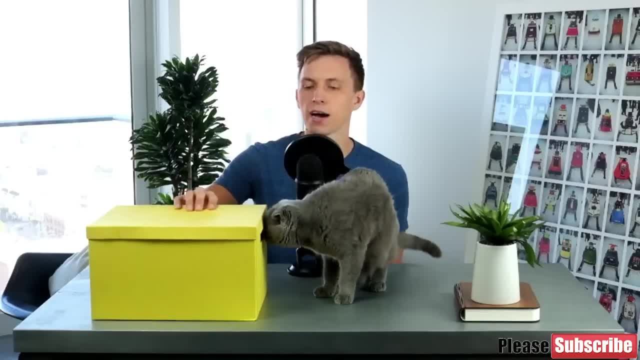 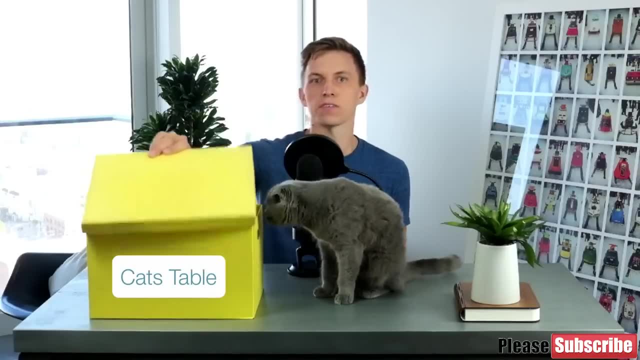 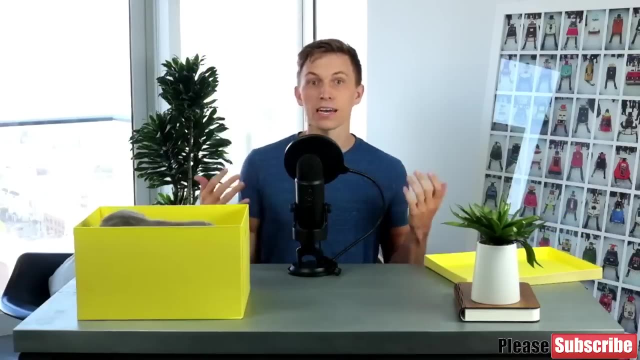 to create tables which are currently empty, to be represented by this Box here. Let's say this is a cat's table, It's empty, It has no data in it, But in this section I'm going to show you the tools to insert data into the cat's table. Thank you, Blue. That was perfect, So we'll see how to do. 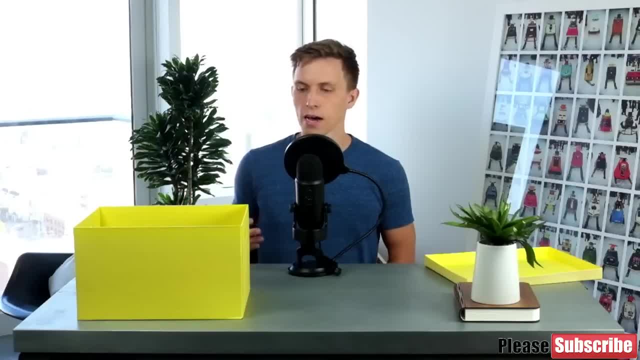 that It's a insert command. So we'll see that and get lots of practice, lots of exercises inserting data into tables. And then the other thing we're going to see in this section- it's not the primary focus, but it's. 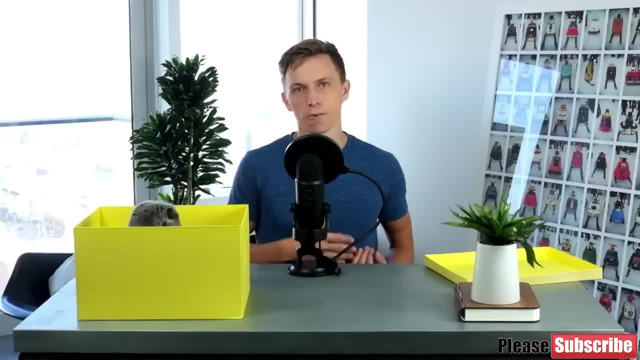 important is selecting data back out, And I won't remove Blue from the box just yet. She's very paranoid. She loves this box, But the idea is, rather than deleting things- that's for another time, another section- How can we retrieve it out? How can we read it or search? So let's say, insert I. 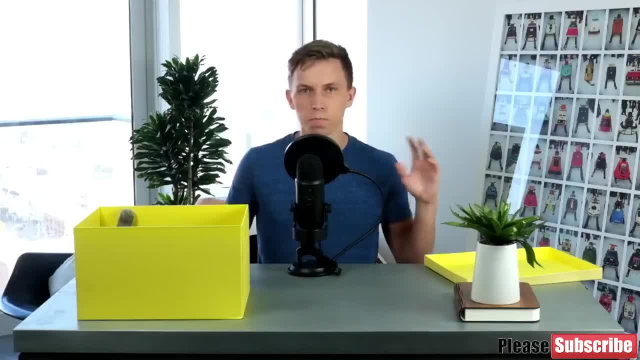 don't know 10 cats into a box And they all have different birthdays and breeds and names. I want to be able to run code like select or retrieve the last five cats added or retrieve the names of the cats that are in the box, And then I'm going to 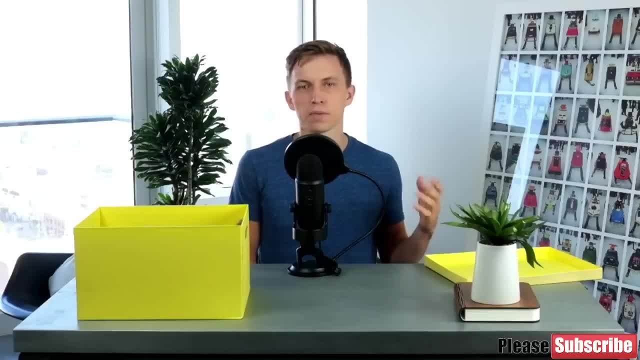 retrieve the names of the Russian Blue cats or retrieve the names of the last, I don't know, the oldest cat in your database, something like that. Wow, she's having a lot of fun in there. So that will be. the goal in this section is to show you those two. 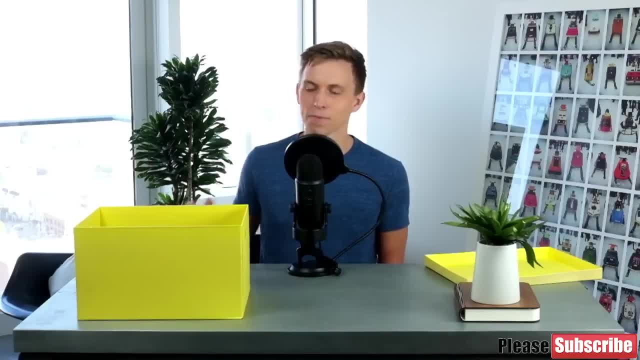 commands inserting data and then retrieving it back out. I'm just going to leave her in there. I can't stand to take her out. All right, well, I'll end it there. Blue's enjoying her box. I'm enjoying whatever this is Next up, we're going to focus our 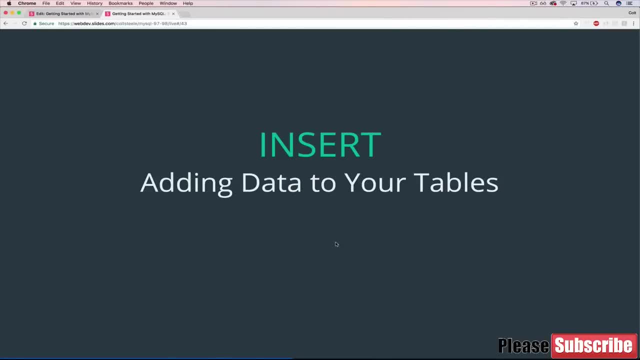 Next up we're going to focus our Next up. we're going to focus our time on learning to create data. How do we add or insert data into the tables that we've already made? This is another one of the most important and most commonly used commands. when you're working with databases, Obviously, it's really important to have a way to get your data in the database. So we'll be using what we learned here throughout the rest of the course- And you could say that for everything else that we've learned so far- but in particular, this command: insert, or insert into. 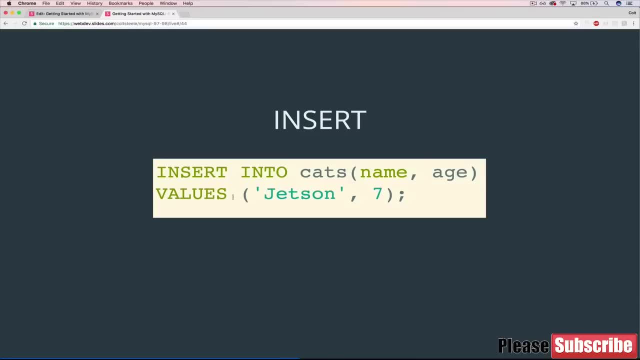 So the syntax here is: insert into and then the name of the table- cats in our case- And then it gets a little weird after that. So let's just focus on that: first insert into and then the table name. Then afterwards, in parentheses, we're specifying the columns that we are going to insert. So I'm saying I'm going to give you a name, comma, I'm going to give you an age, And then down here I have values. 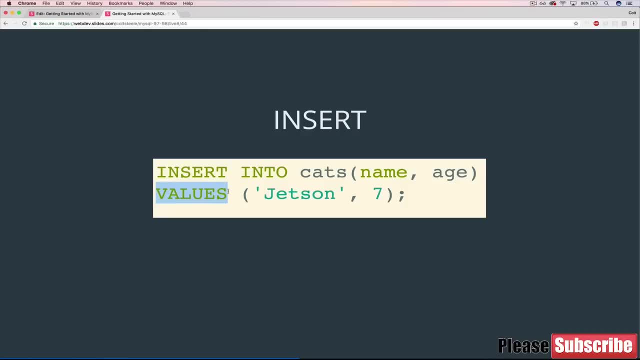 which is another keyword specifying that. okay, I told you, I'm giving you a name and an age. Here they are: The name is Jetson and the age is seven, So these do need to match. Name is first Jetson. 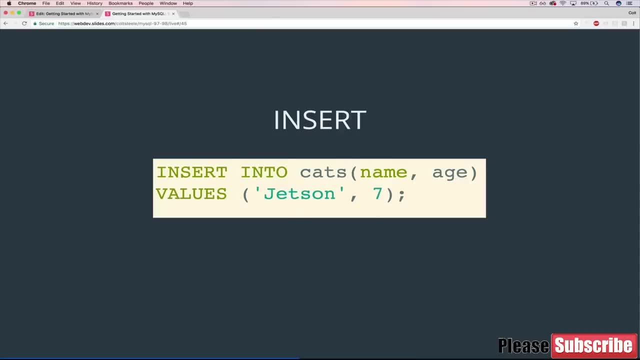 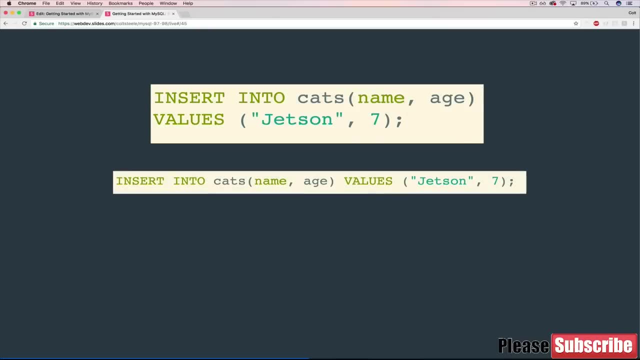 age is second seven. Before we go try it out in Cloud9, I just want to show you that I wrote it this way mainly because it looks best on a slide. You can do it on one line, So insert into cats name and age values, Jetson and seven. or you can do it like this, And this is actually a lot. 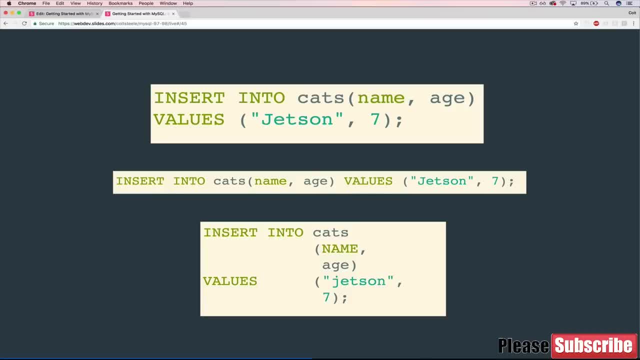 of people's preferred way of writing it, But this is a huge pain to enter into the shell this way, where you have to space things manually. But when we start working with individual SQL files where we'll save our own code basically into these separate files in a text editor. 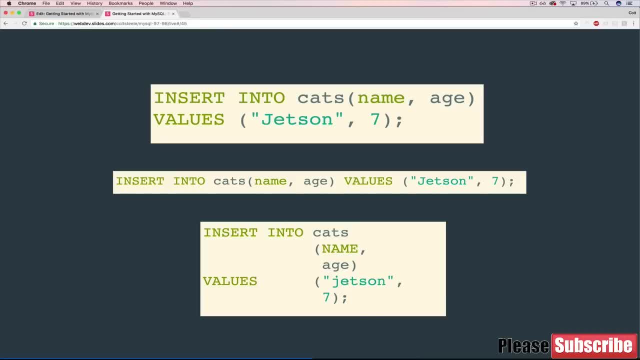 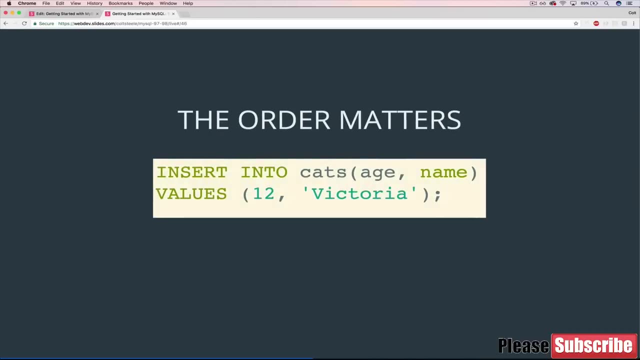 and we can space them out how we want. This is definitely a preferable way, But we're going to work with this. I just like this when I'm presenting and when I'm teaching it. It's a mix of readability, but also it's not so laborious like this. Okay, And just to hit this point home. 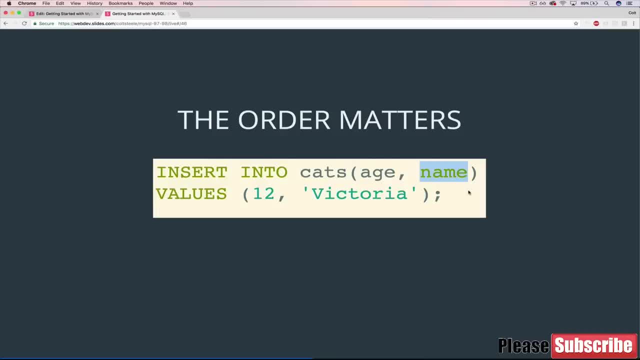 the order that we write these column, names matters. So if I say insert into cats and I say age is coming first and then name, I have to provide age first and then name. So it doesn't matter which order you use, but whatever you establish, 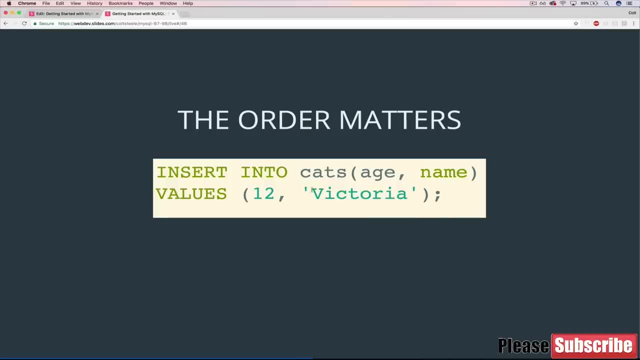 up here you have to follow through with, Otherwise it will try. if you had this reversed, it would try and assign Victoria to age and 12 to name. And that's going to be a problem because we have these strict data types where things are supposed to be numbers and strings, And so if we 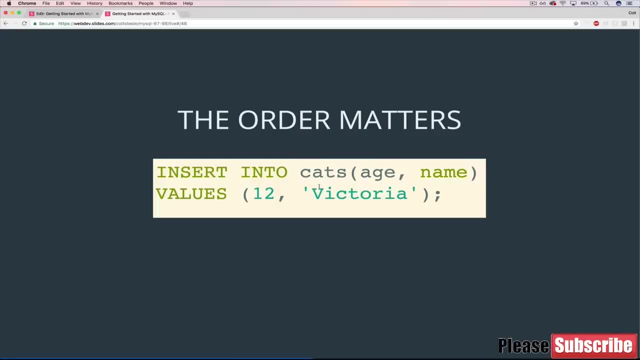 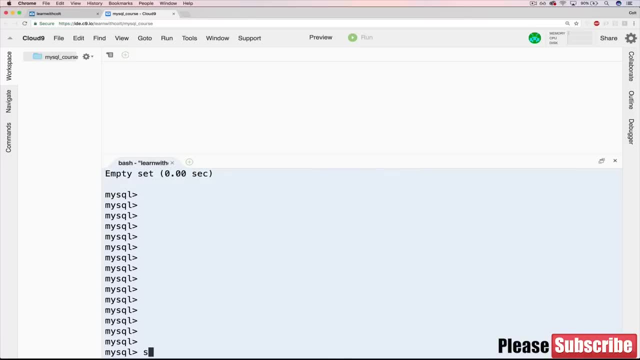 mix them up. it's problematic, Not to mention that it makes no sense. So let's give it a shot in Cloud9.. I'll make some space here, And the first thing we need to do is actually recreate a table, because right now I don't have a cat's table. I deleted it because I showed you how. 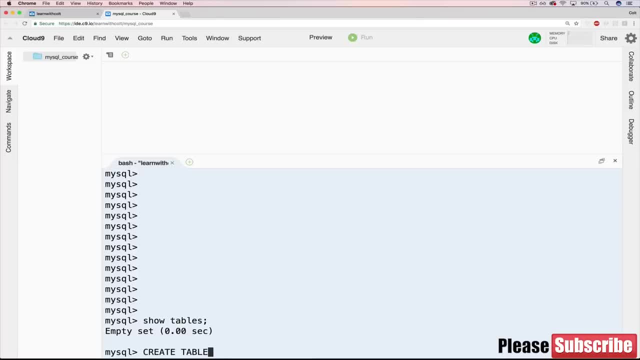 delete works. So let's recreate that, Create table cats, And it's going to have name, So varchar, 50 comma age is going to be an int, Just like that. Perfect. So now we'll use the insert into command. we just learned, So we will insert a new cat Insert. 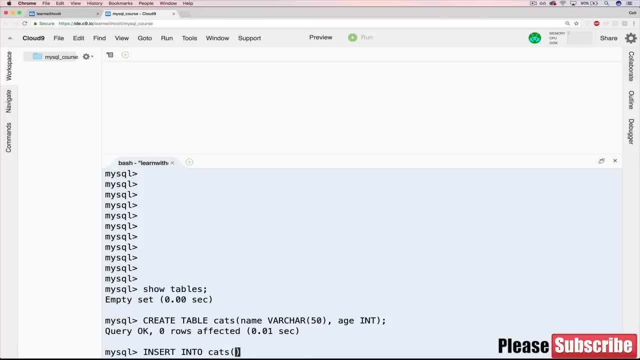 Into Cats And I'll start with name And then age, And then I'll go to a new line. I don't have to, but I like to. Values And the values we'll put in, let's say, for name, let's work with my cat. 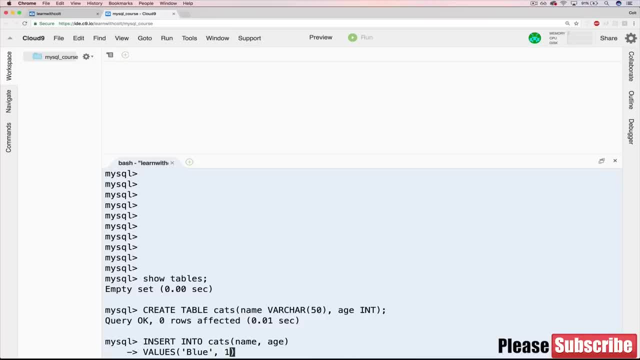 blue Comma And her age is somewhere between 1 and 2.. We'll just leave it as 1. Semicolon, We'll hit enter. We get our query okay. This time it says 1 row affected. You may have noticed that everything else we've done so far. 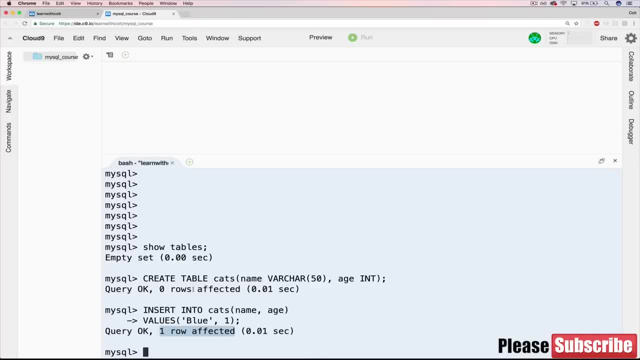 has said 0 rows affected, And I think that's pretty self-explanatory. We haven't had any rows of data yet, So all of these commands have returned 0 rows affected. Now we actually have created something. We've added data to a table And it says 1 row affected. And before we move, 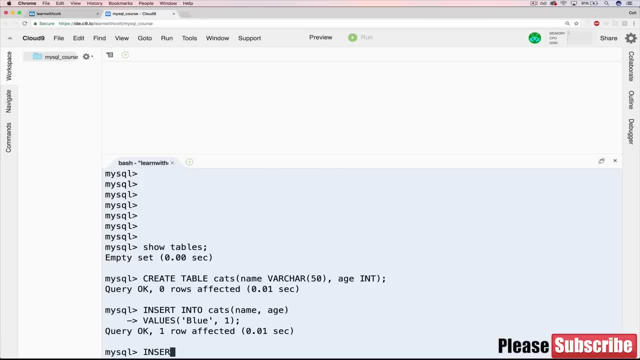 on. let's insert one more cat here, And this time we'll switch up the order Insert into cats And we'll add one line: Age, comma, name And then our values. Let's say the age for this cat will be. 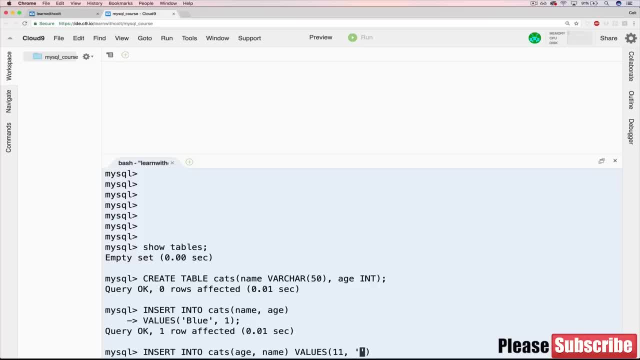 11. And the name will be Draco, All right, And we also get 1 row affected. So next logical question might be: how do I see the data? How do I know that it's in there correctly? Basically the same thing that you might have asked when we saw how to create a table. 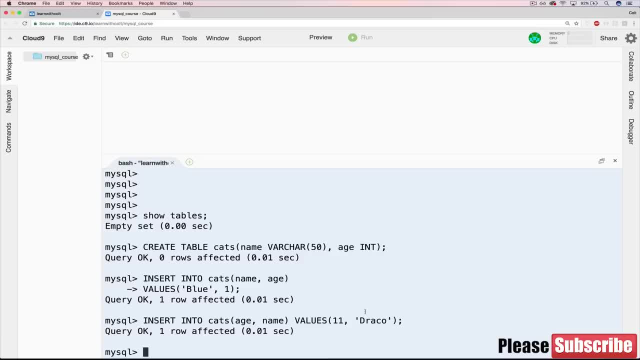 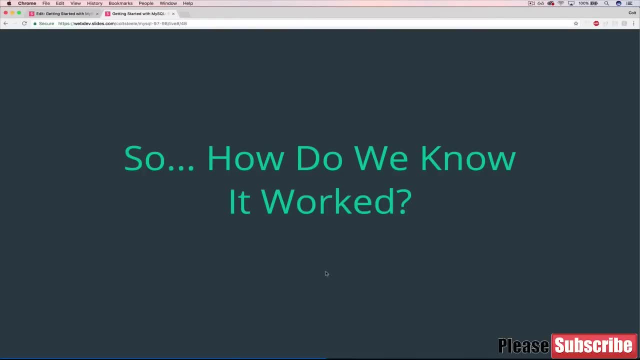 How do we check our work? Well, we've created data in a table. How do we check our work? And we'll see that in the next video. Sorry for the cliffhanger. Okay, So we left off with a little cliffhanger, which was: we've inserted data, How do we know that it actually worked? And the main, 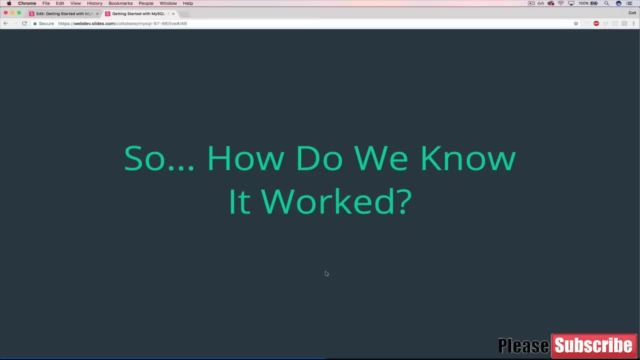 reason I made this a separate video is that it gives me a few seconds, a separate opportunity to talk about one of the main dilemmas behind figuring out how to best teach this content, which is that pretty much everything in this course is related And interdependent, or a lot of it is. So here's an example I'm showing you I'm talking about. 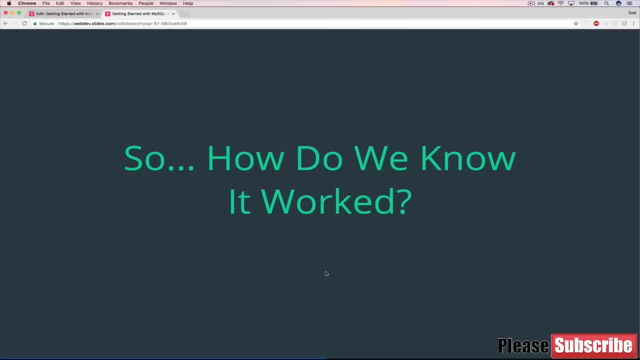 inserting data. but it's really not that great of a learning experience unless you know how to view data. But if I teach you to view data first without having you insert it, there's nothing to view, and so on. So my approach is to try and teach things in isolation but then kind of bridge the 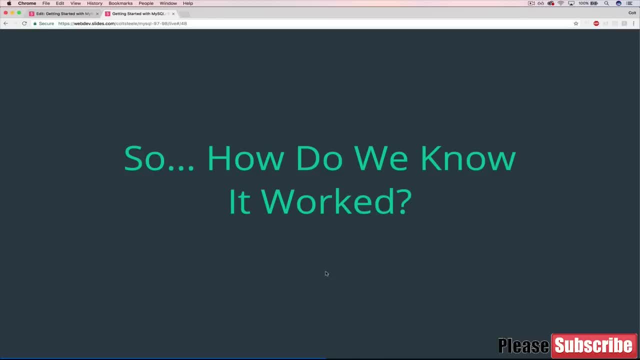 gap and give sneak previews when necessary. So, with all of that in mind, I'm going to show you a little bit more of a tutorial that's coming up in the next section. So, with that said, I come from the future here. with SQL command, you won't actually learn- learn officially- until the next. 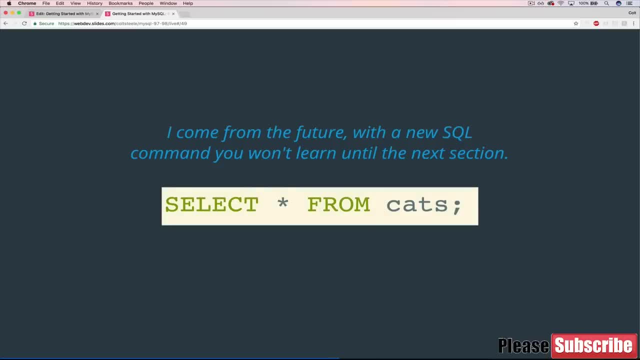 section. So for now you can just copy this. We we're not going to talk about really what it does or how it works Until the next section. we'll dive a lot more into the select statement. But to view all of our data in any given table, select star from the table name. So select star from cats. 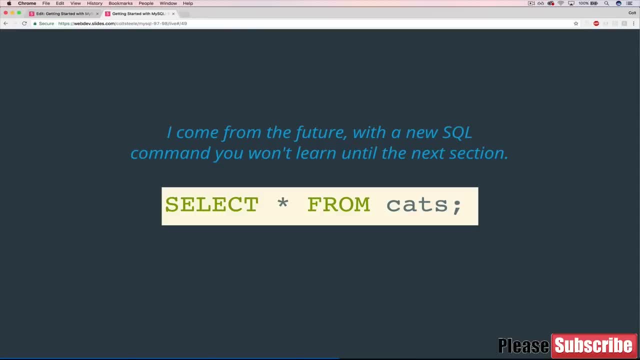 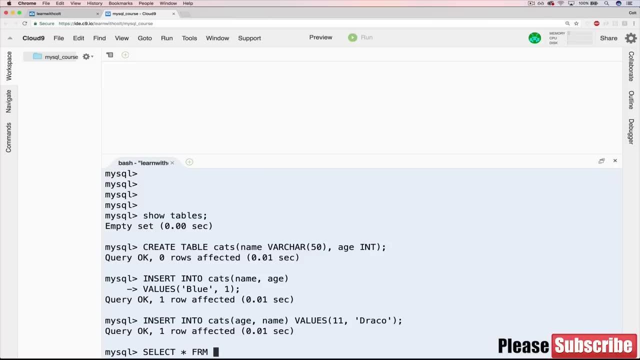 And that's all I'm going to say about it inserting data. This is just going to help us check that it worked, So let's try it. We should have two cats in there. Select star from cats And there we go. We've got name and age, We have blue. 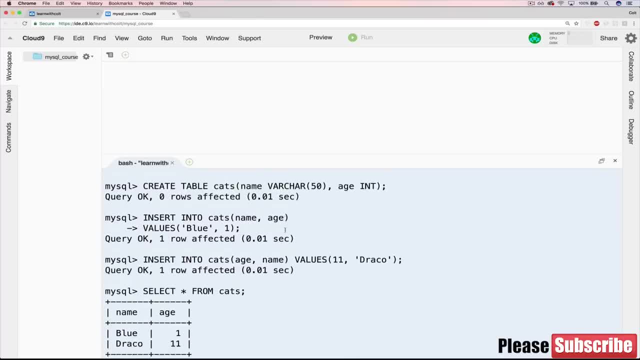 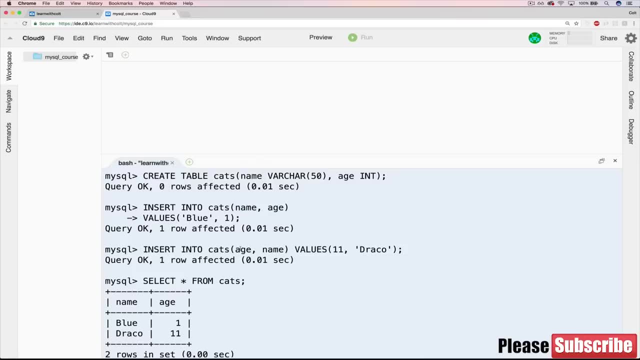 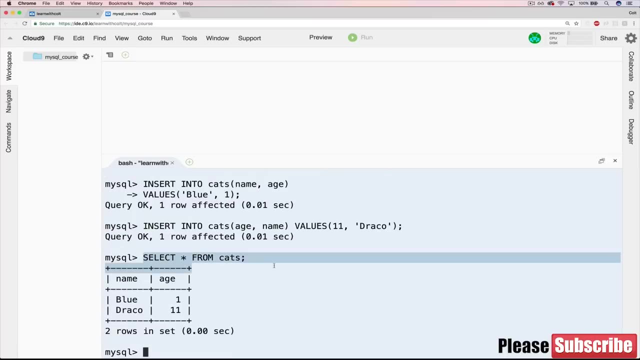 who is one, and Draco, who is 11.. And remember, we inserted these in different orders, So we did name and then age for blue, And then we did age, followed by name for Draco. So that's all there is to this. We know that it works. There's a lot more to using the select command, Probably 30% of. 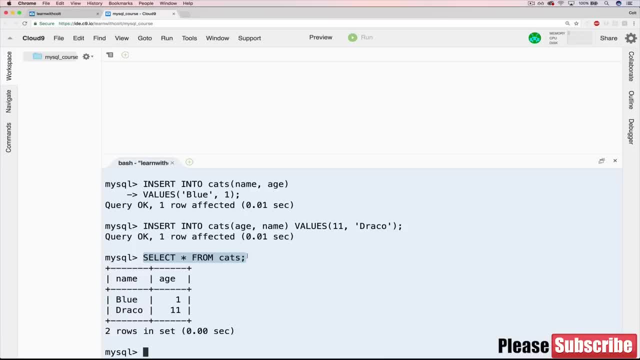 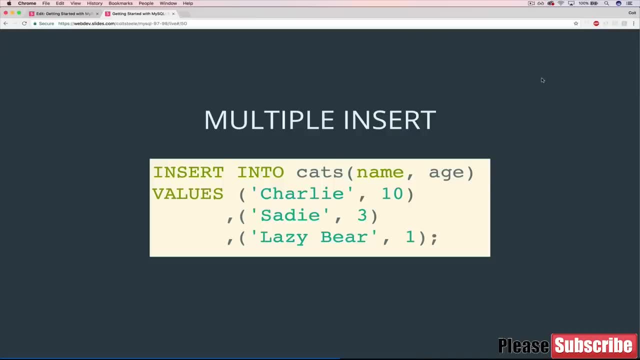 this course will be focused on selecting data and filtering and sorting and searching and all sorts of different ways of viewing data. But for now this is a magic little shortcut. So another thing to know about the insert command is that you can use it to bulk insert data, So we can insert 10. 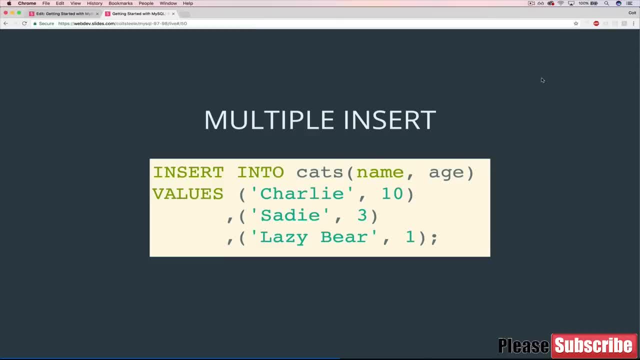 different users at once, Or we can eventually, once we get to it, we can update 10 different users at once or delete 10.. Or whatever it is. But for insert, the way that it works is that, rather than just giving one set of 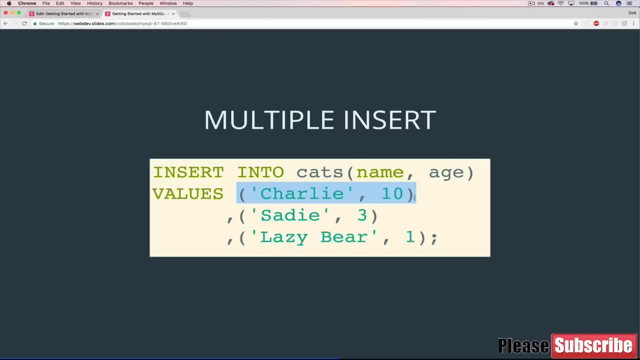 values, like Charlie, who is 10, we just use a comma separated list. So we tack on a comma and then we add another one, Sadie, who's three, and then comma lazy bear, who is one. A note about the comma. 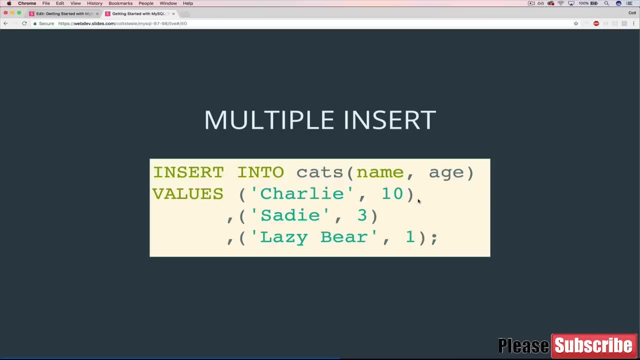 placement does not matter, You'll see it. I think what's more logical is actually to put it here at the end of the line, But often what you see is here. I think it makes it easier For you to just visually break things up and to see: OK, here's a new line and here's a new line. But 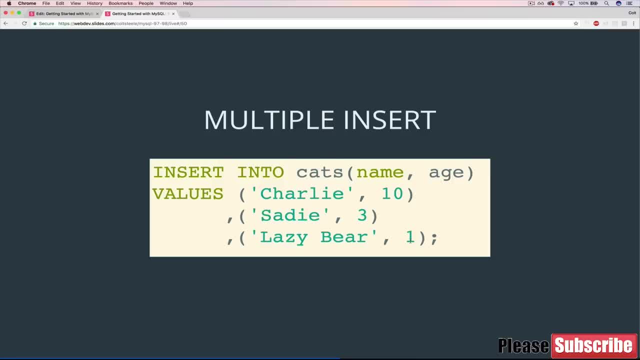 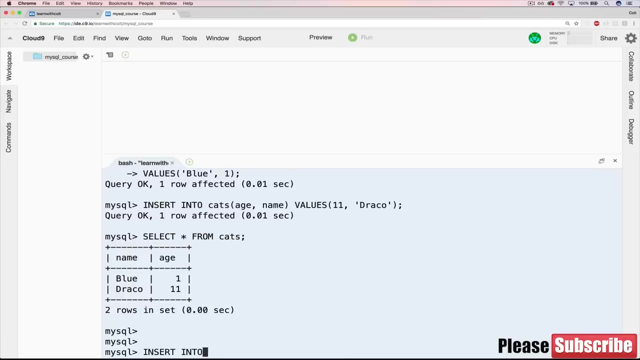 really just a matter of preference. So don't pay too much attention to that. Don't pay any attention to that. actually, What's important is that we have a list And we can multiple insert all at once. So let's try it. So we have our cats table with blue and Draco. We will do an insert into cats And we'll do name. 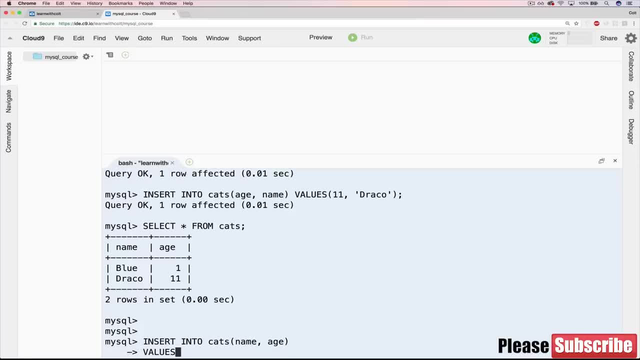 followed by age. Now we have values And our first pair or our first set of values will be: oh boy, this is the hardest part of teaching this stuff: coming up with the fake data. Let's say peanut And peanut is two And comma. You could have put the comma there, It doesn't matter. Let's say the next one will be called butter. 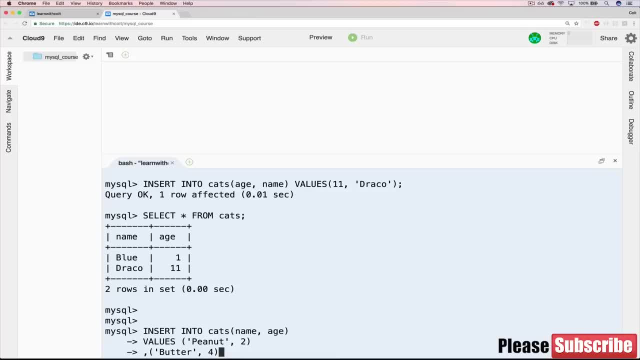 Who is four? Yes, I am looking at a thing of peanut butter in my kitchen right now, So that's where that comes from. And lastly, let's do sure, jelly. Who is seven? Just like that, We need our semicolon to end it. 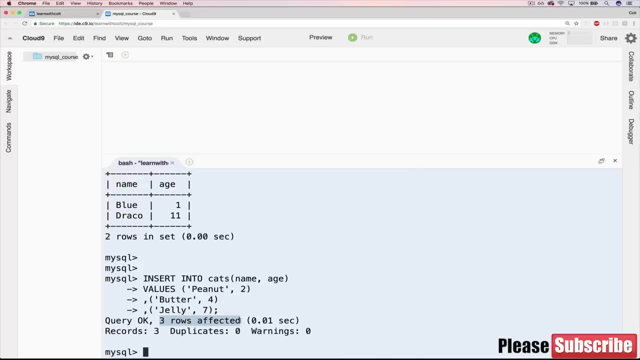 Now we get something slightly new. Query: OK, three rows affected, Awesome. So to check our work, we can just do select star from cats again, And I should be consistent. It doesn't matter, but I'll capitalize the from Now we have blue Draco, which were there before peanut butter and jelly. 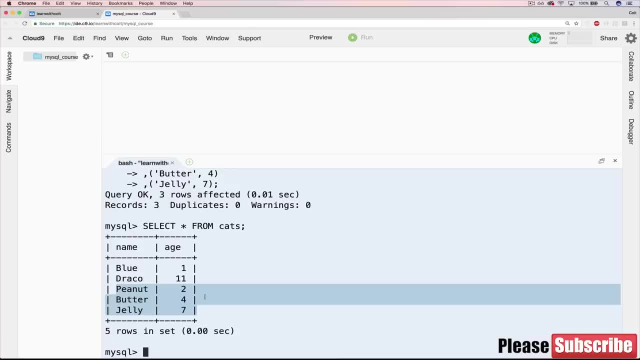 That turned out nicely And we inserted them all with one command. So later on in the course, when we start working with some more complicated data, what I'll actually do is give you a file that has an insert statement that will insert, let's say, 20 different items into a database- 20 rows. 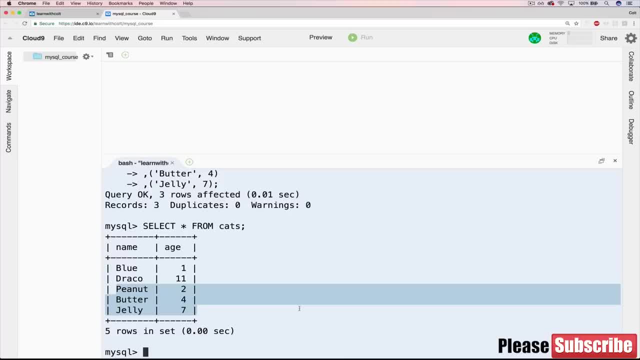 And you'll be able to run that one line and get kind of starter data that you can use. It'll be an easy way to populate your database with data without having to do it manually 20 times. OK, so that's all there is to multiple inserts. 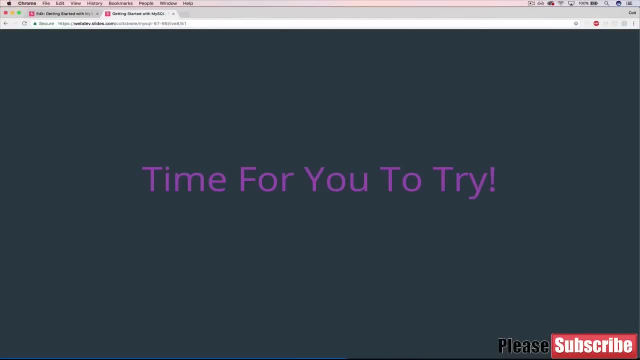 All right, so it's now your turn to give this a try. You're going to get some practice using the insert command, So we'll be working with people. this time You're going to create a new people table, So actually, this is going to combine both creating tables and inserting data. 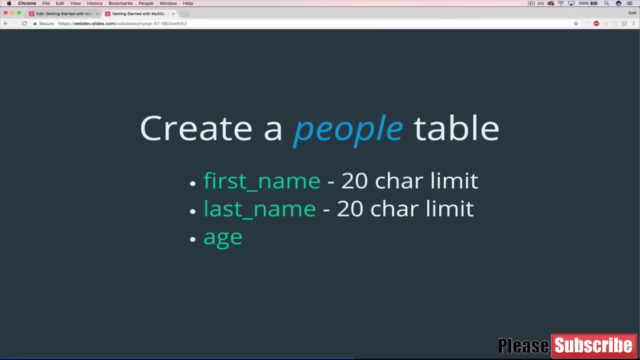 So the table you'll need to define will have three columns: First name- that has a 20-character limit. Last name also has a 20-character limit. And age, which is a number. So once you've defined that table, the next step is to insert. 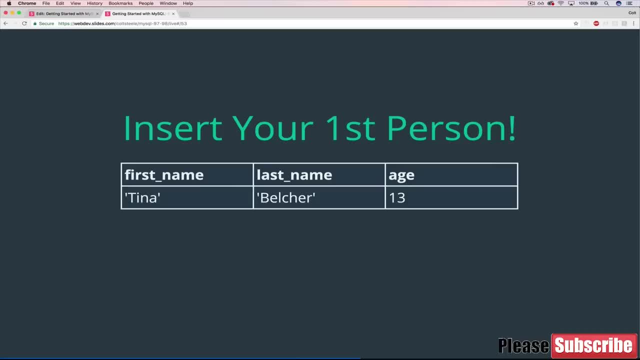 your first person. And for this person, her first name is Tina, Her last name is Belcher and her age is 13.. So once you've inserted her, make sure that you've done it correctly. Use that select command to see what's happening. 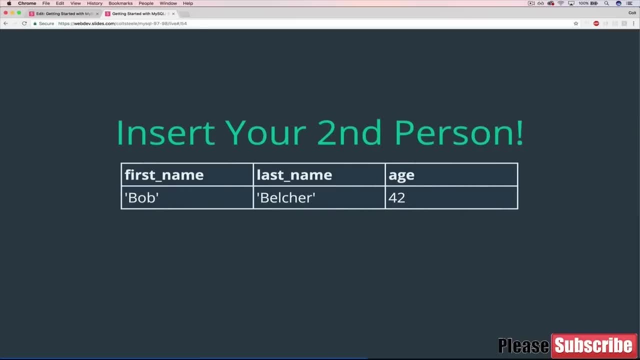 Make sure she's in there. The next person will be Bob Belcher, who is 42.. And it's up to you, but I would like for you to try and insert this one using a different order for the values. So if you had said: 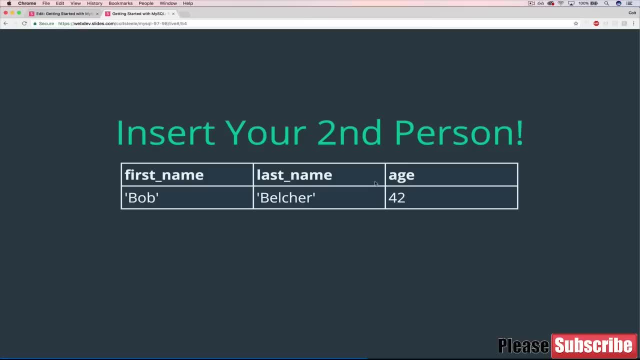 first name comma. last name comma age. in the previous one maybe try last name comma age comma first name. Doesn't make a lot of sense to do it that way, but give it a shot, just to prove that you understand that the order matters. 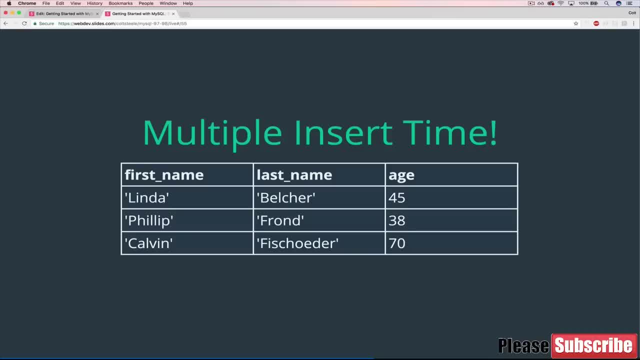 And then lastly, write one insert that will insert three different people at once, And that will be Linda Belcher, who's 45,, Philip Frond, who is 38,, and Calvin Fishoder, who is 70. So insert all three of those at once. 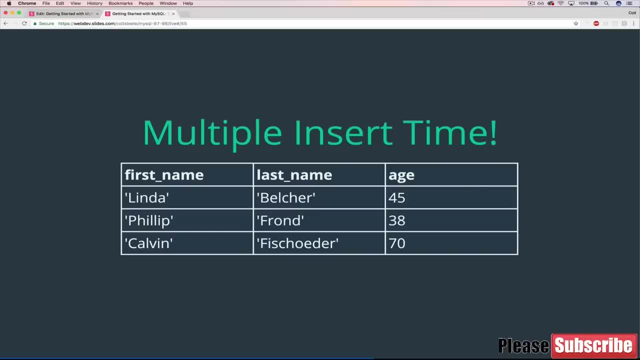 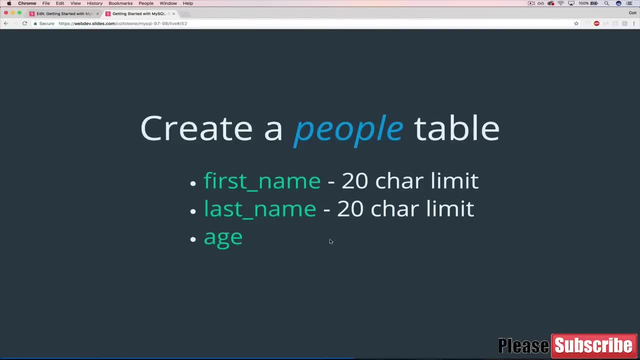 And go ahead and give it a shot And in the next video we'll have a solution. OK, let's take a look at a potential solution for this people problem. So, first thing, we need to create the table using the create table statement. 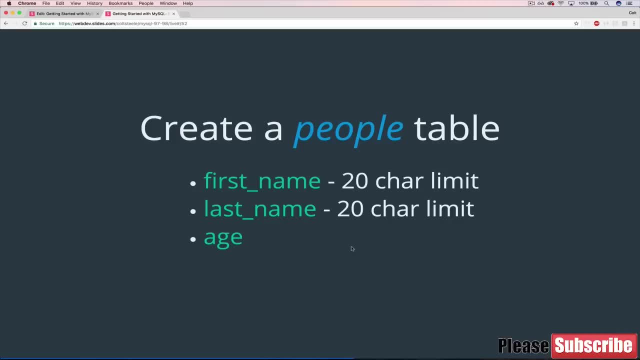 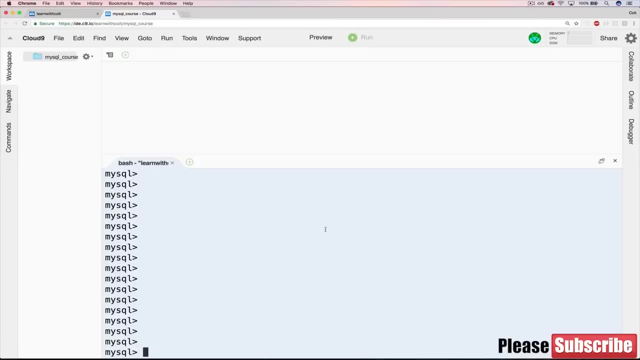 with first name as a varchar 20, last name varchar, with a 20 character limit and age as an int. So let's do that. I'm just working in the Cat app for now. It's fine, We're going to delete this at the end. 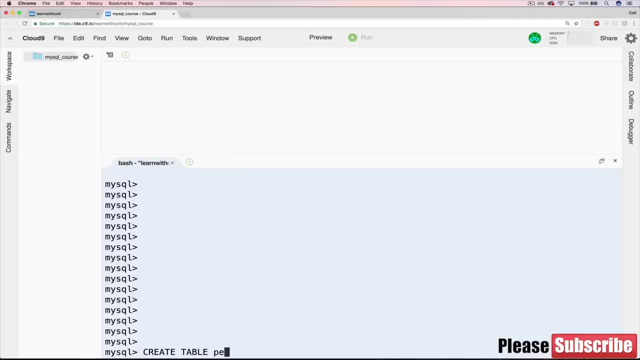 So we'll start off with the create table And we'll call it people, And the first thing that we'll have is first name, which is varchar 20.. Next thing is last name, which is the exact same, And then, finally, we have age, which is an int. 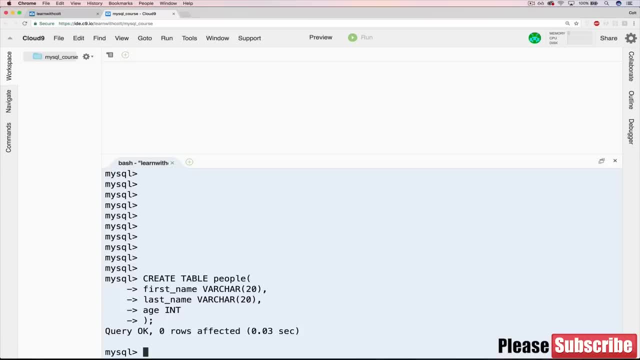 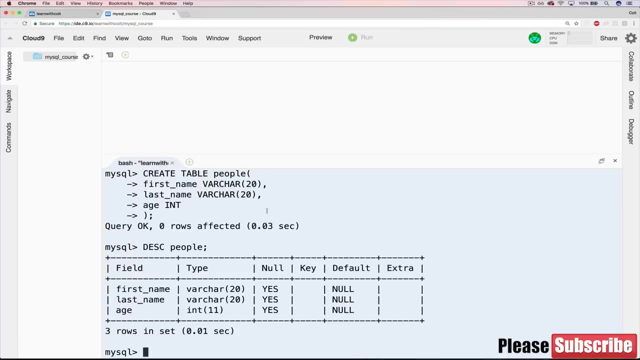 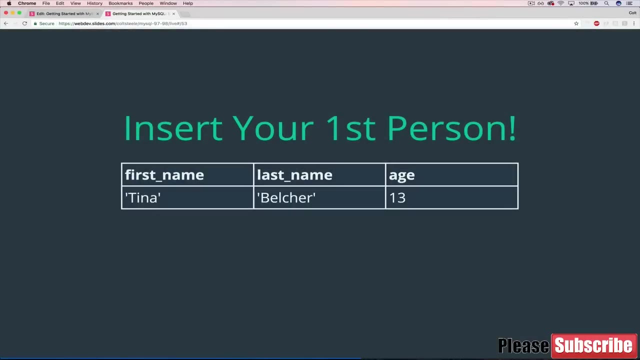 And that's it. And then our closing parentheses. OK, let's just double check. it worked. Let's use describe people: Cool. First name, last name, age: varchar, varchar, int. Perfect. So now we're going to insert our first person, Tina Belcher, who is 13.. 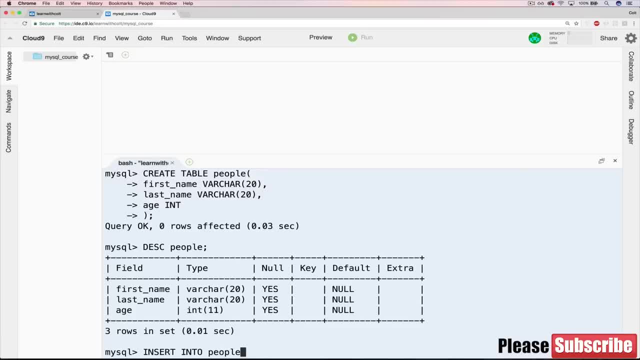 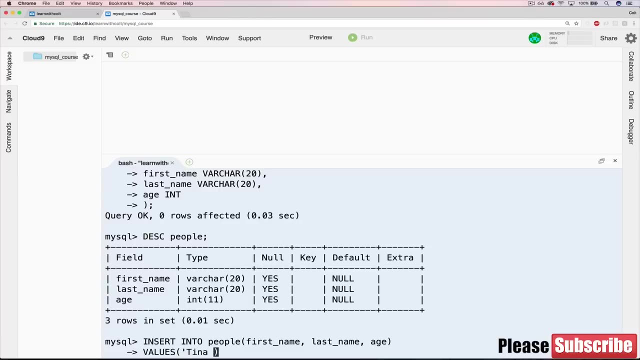 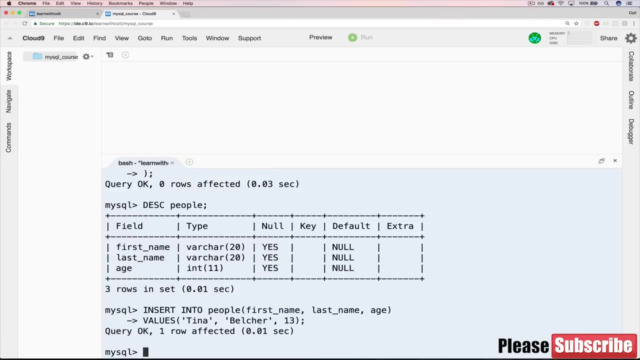 So insert into people And we'll start off. Let's do first name, Last name, age And then values And we'll do Tina Belcher, It was 13,. right, OK, We hit enter. Just double check that it worked. 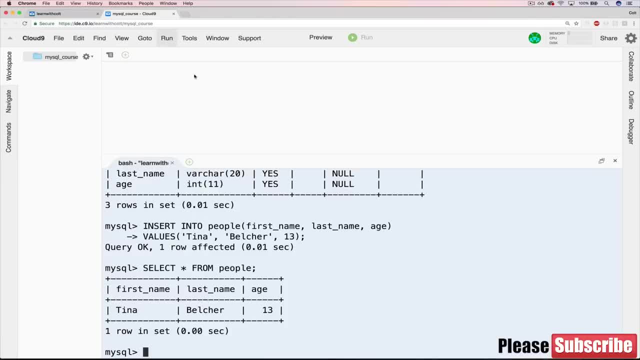 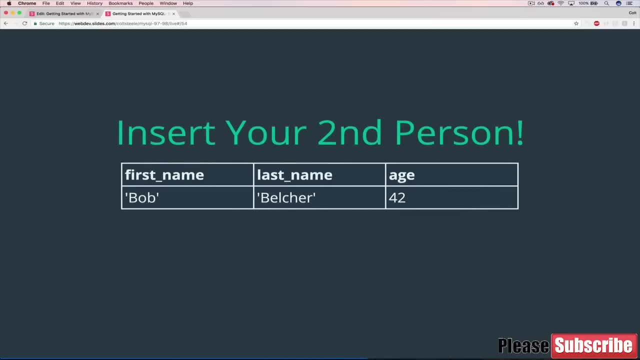 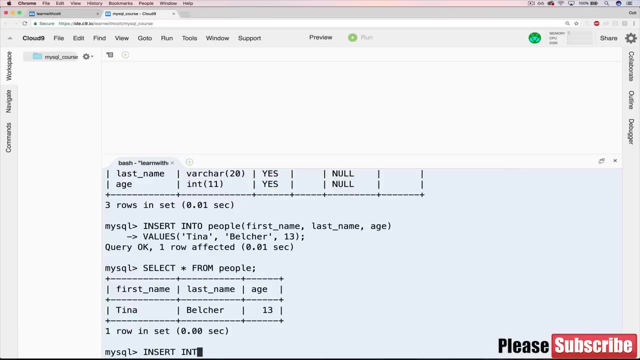 Select star from people There. Tina is perfect. Now we're going to insert our second person, Bob Belcher, who is 42.. And my instruction here was do it in a different order, So we'll do an insert into people. 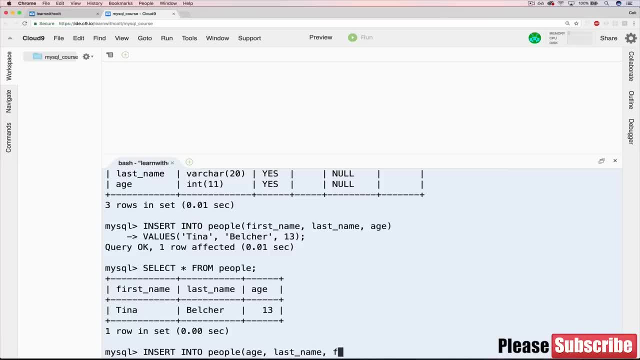 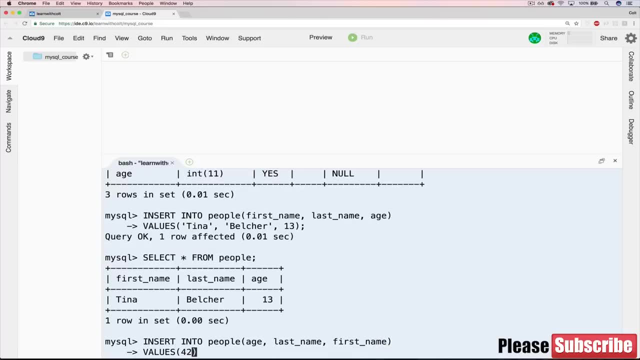 This time let's do age. last name, first name Values. So age was I already forgot Jeez, Last name is Belcher And first name is Bob. Don't forget our semicolon. Let's do our select again. 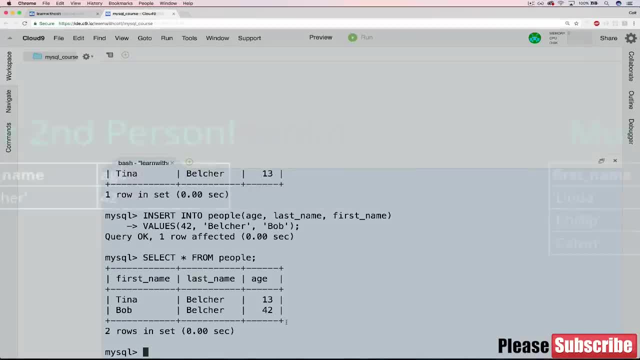 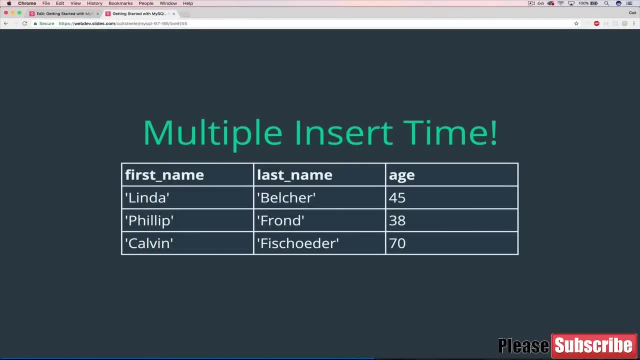 Perfect, It worked out how it was supposed to- Great. So then, the last insert we're going to do is a multiple insert. We have Linda Belcher, Philip Frond and Calvin Fishoder. Oh boy, This is going to be a lot to remember. 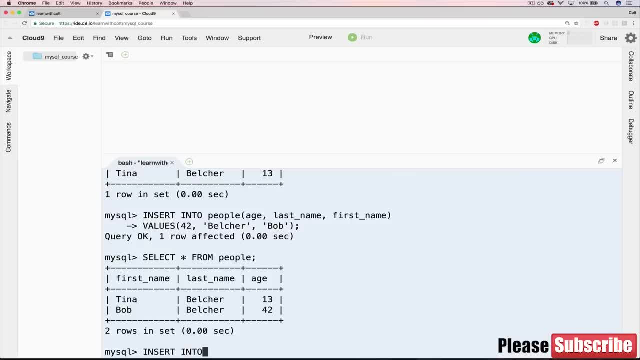 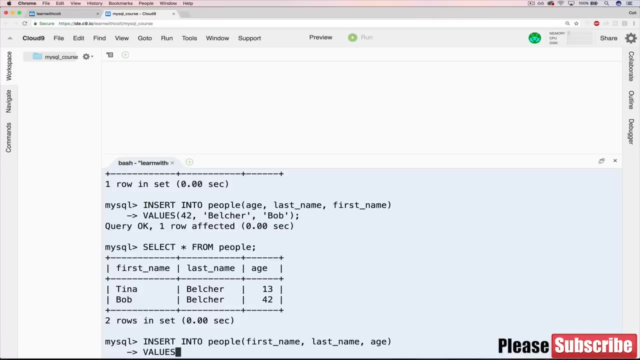 Let's start off by just typing out the basics- Insert into people- And we'll do this one with first name, then last name and then finally age, Just like that. Then we'll do values And we'll start off with Linda Belcher, who is 45, I think it was. 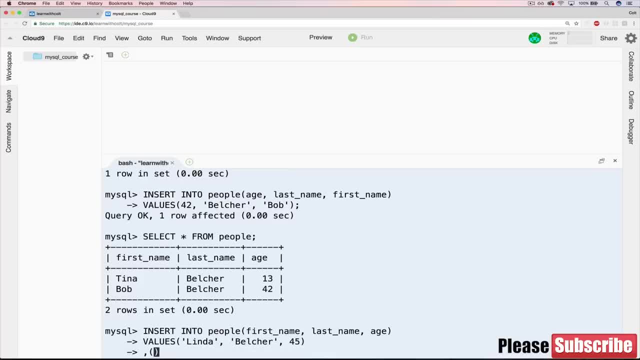 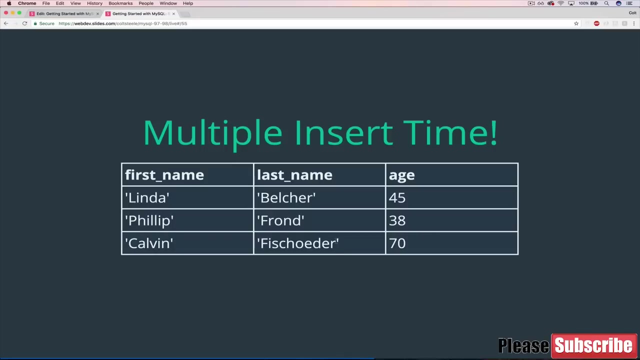 And I'll do commas on the new line And then we'll go. Then we'll go with Philip Frond, And he is 45.. No 38.. I made this too hard. Lastly, we have Calvin Fishoder. I'm just going to copy Fishoder, who is 70. 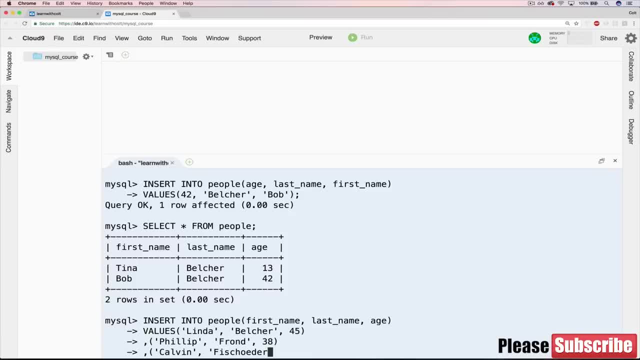 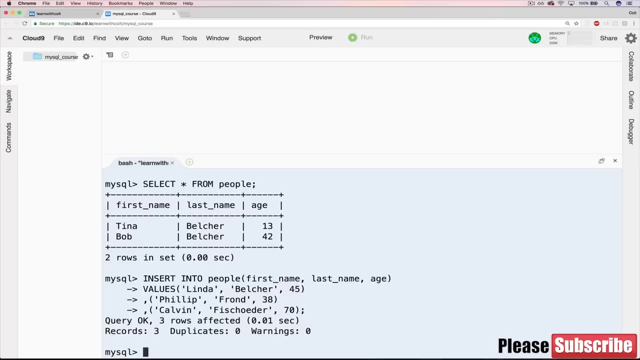 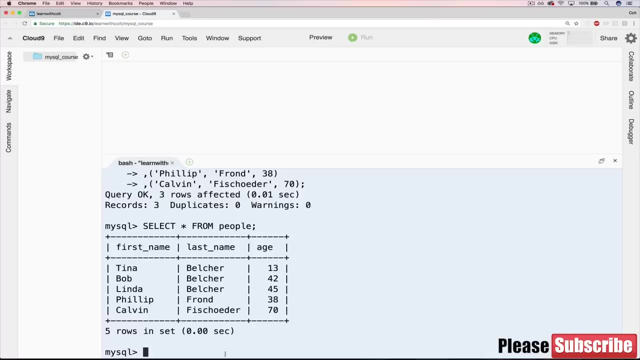 Calvin. Okay, Calvin Fishoder: 70.. All righty, And before I forget, we need a semicolon Perfect. Let's do our select star again. I have to use the up arrow a couple times And we have Linda Philip and Calvin Belcher. Frond Fishoder: 45,, 38,, 70.. 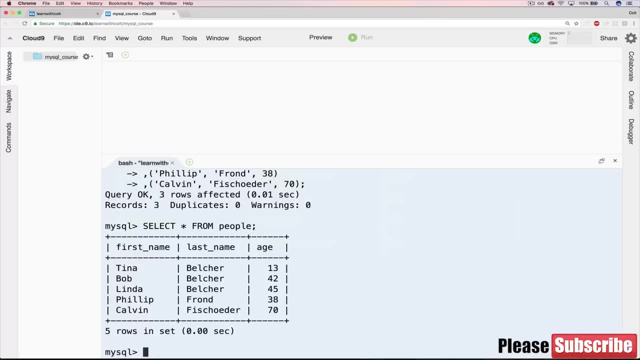 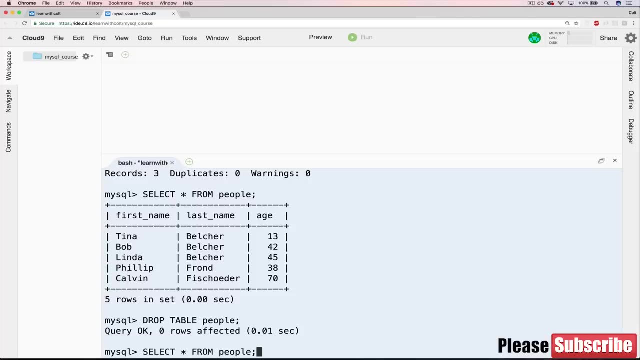 Perfect, So that's it, And I didn't specify this in the instructions. but let's go ahead and delete the table. So that's drop table people. Goodbye to the Belchers and the other two, And we verify that it's gone. 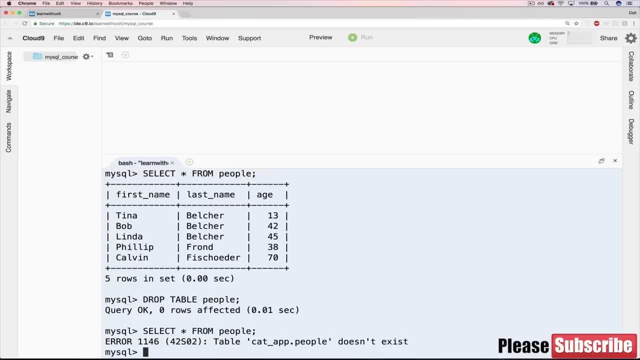 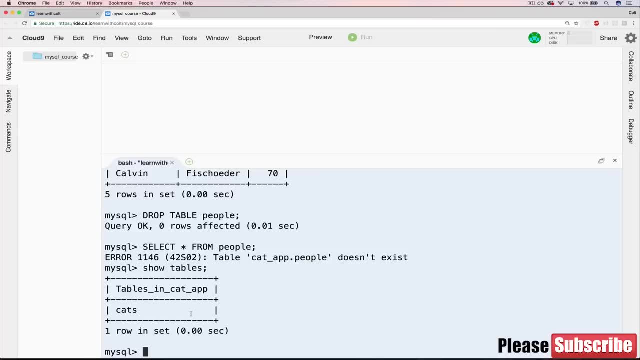 If you tried to do select star from people, we get an error. But if we do show tables now, we only have cats. All the people are gone, just left with cats. Now this video is going to be a slight departure. 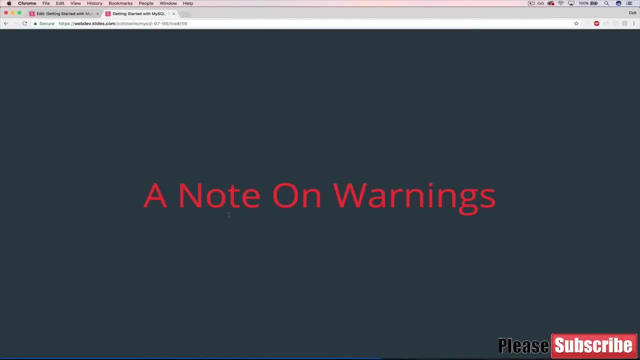 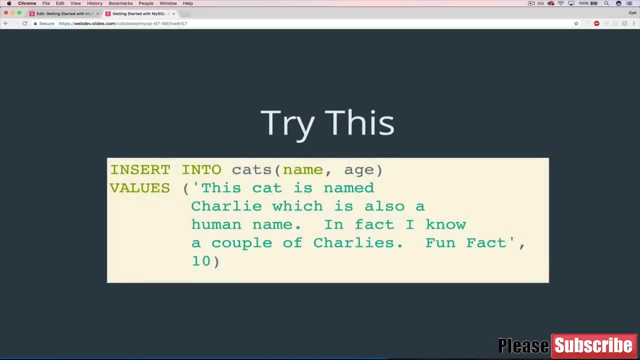 We're still working with inserting data, but it's a slight side note Which has to do with something called warnings. So, to illustrate what I'm describing here, if we tried to insert something that looks like this: So we're going back to cats. 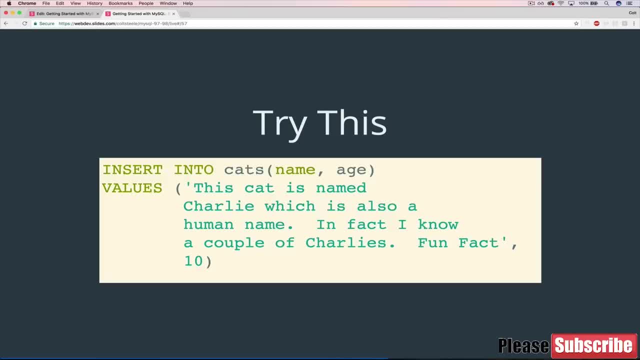 And our cats have a name and an age. If we tried to insert a cat whose name is this gigantic string, This is a cat named Charlie, which is also a human name. In fact, I know a couple of Charlies, Fun fact. 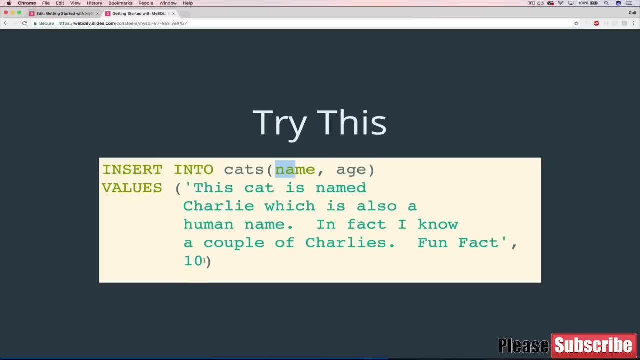 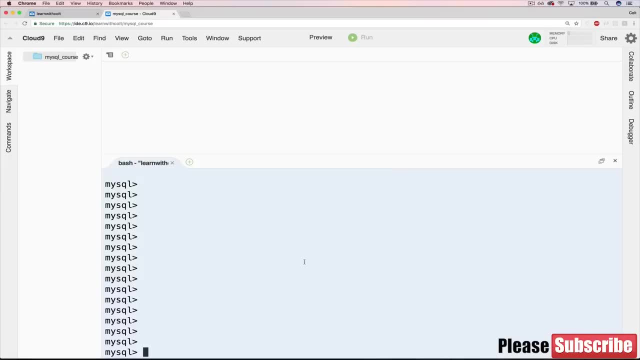 If we're trying to put that as this cat's name, an age is just 10.. If we do that, Let's go ahead and copy this, just so I don't have to type that. Make sure we have our cats table. 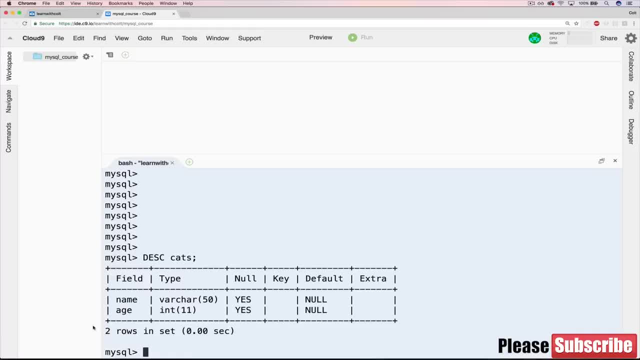 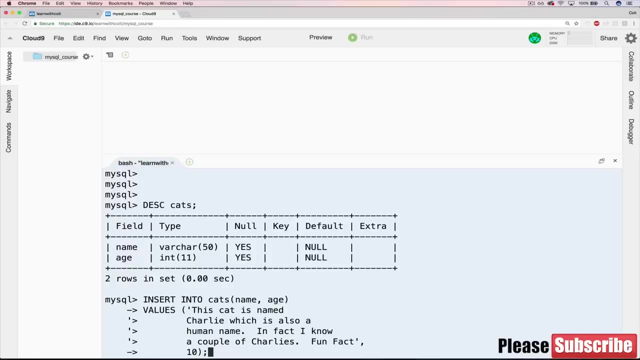 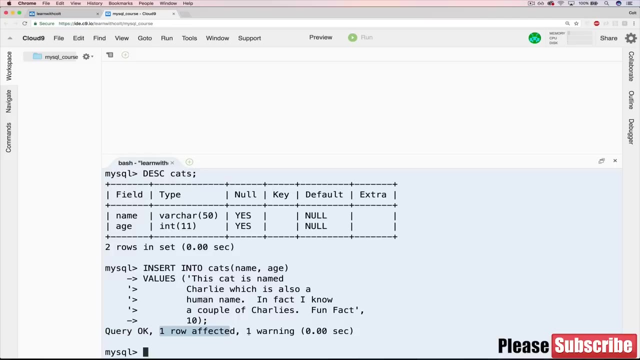 Let's do describe cats, Okay, so name and age. Remember there's this restriction here of 50.. I'm just going to paste that and put a semicolon. I get something that says: query okay, one row affected, one warning. 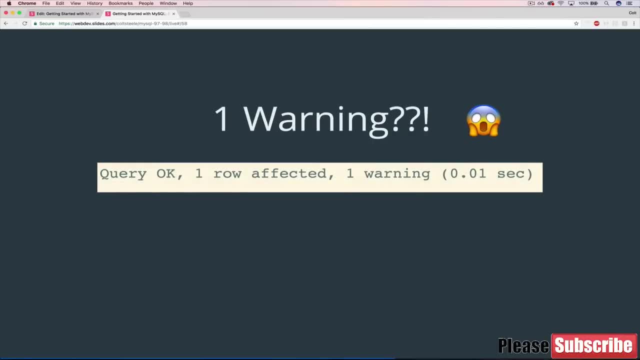 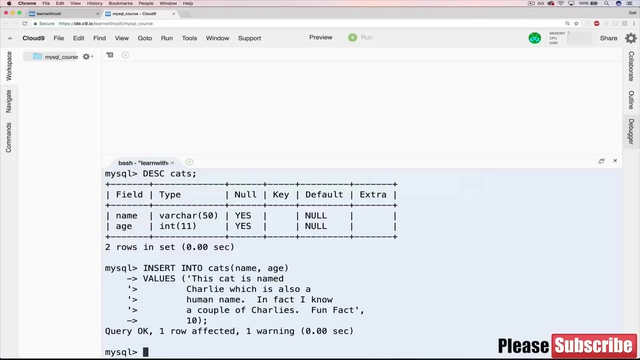 Just to double down on that, I pulled it out into a separate slide. One warning: Oh my gosh, what's going on? Well, if we wanted to know what that warning was, we can use this command: Show warnings. So we'll go back and type show warnings. 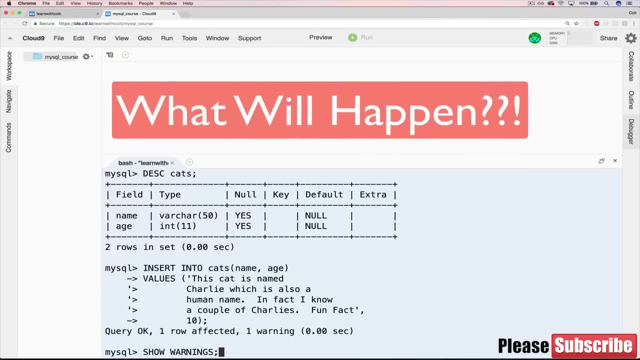 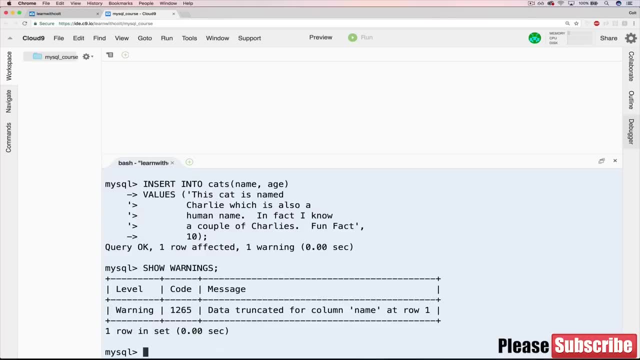 And I want you to pause and think: what is the warning? If you were to guess, Obviously we haven't talked about it yet, But what do you think I'll see? And the answer is: I get a warning here that says data truncated for column name. 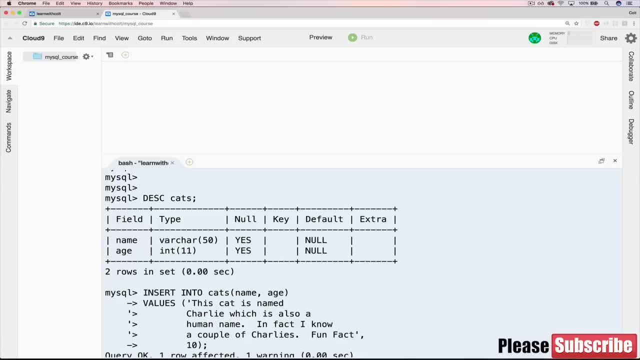 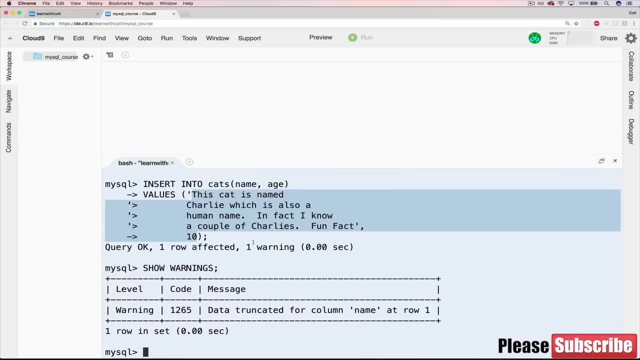 So that corresponds to name here, which had a limit of 50 characters, And this is more than 50 characters. I can't remember how much it is, but it's more than 50.. And if we look at cats, you'll see that our, first of all, our table gets a little messed up here. 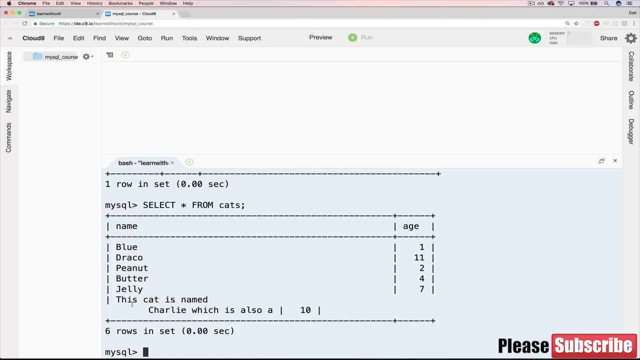 But the string for name gets cut off after this cat is named Charlie, which is also A, And then the rest is gone. So it's not like it's hidden and it's not displaying, It's just not stored at all. So that's important to note. 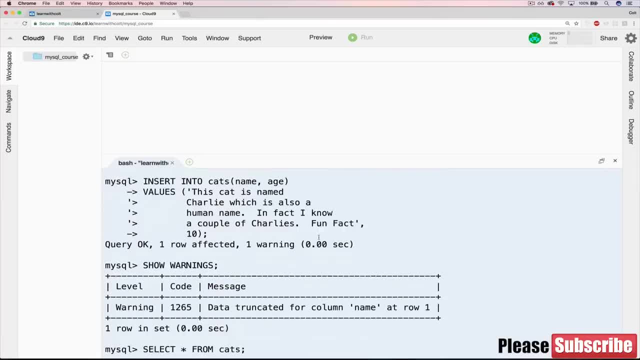 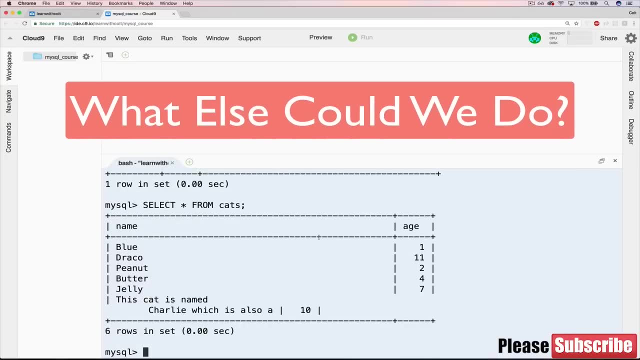 So that's one warning that we saw there, And that happened when our data was truncated. Can you think of another warning we could generate deliberately? What's something we could do that would give us a warning? So pause the video or don't. 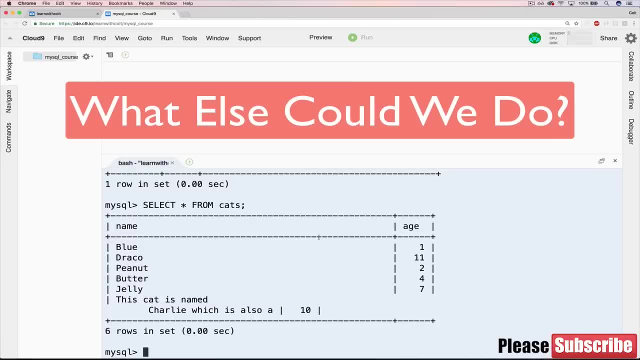 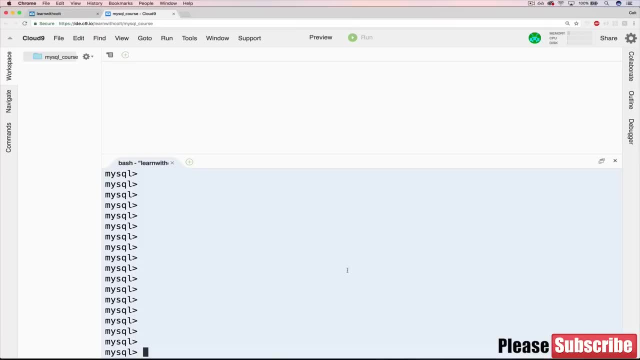 But try and come up with something based off of what we have currently set up for cats. How could we insert something that would give us a warning? All right, So what I was imagining is that we could try to insert something where we mixed up a data type. 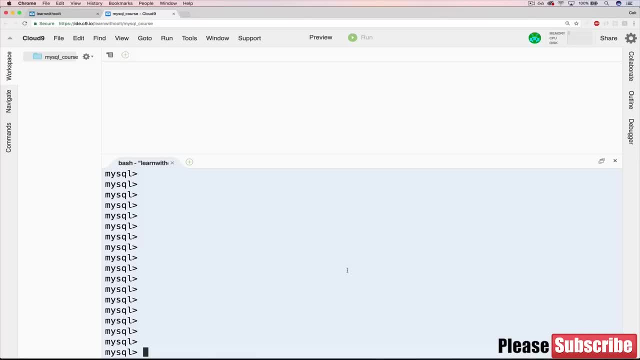 So let's say age instead of being an integer. we passed in some text random gibberish That should generate a warning, So let's try it now: Insert into cats. We'll do name first and then age, And name will just be Lima. 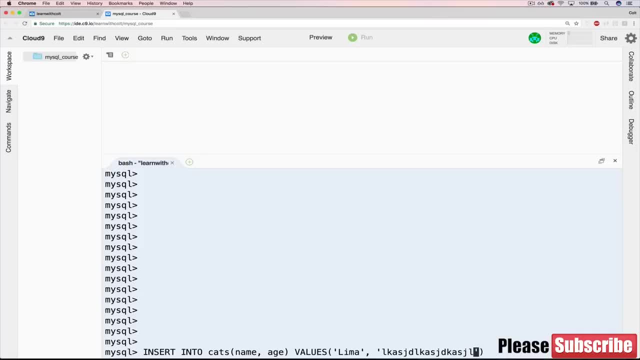 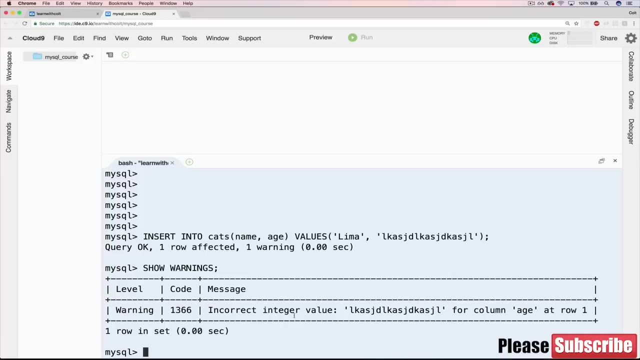 Why not? But age will be gibberish like that, which is not a valid integer value. We'll hit enter. We get one warning And we can view that warning with show warnings, And this time it's a different warning. 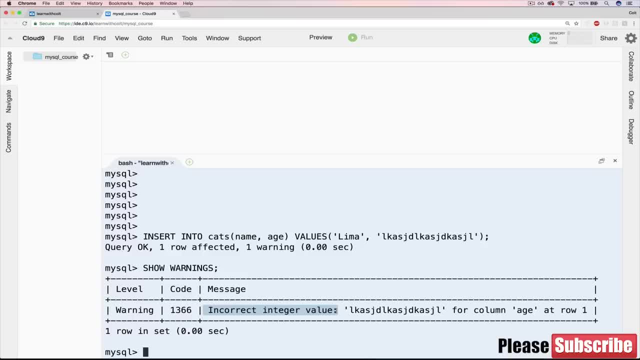 It says incorrect integer value. So the last one we saw said that name was truncated, It was too long. This one is telling us that incorrect integer value for column age. So then here's a second thing for you to think about, And you probably- I mean, you'll just have to guess. 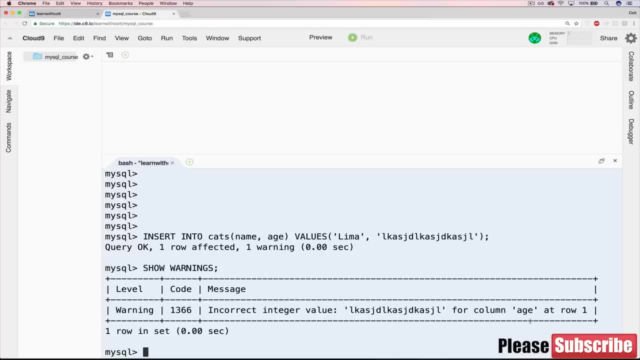 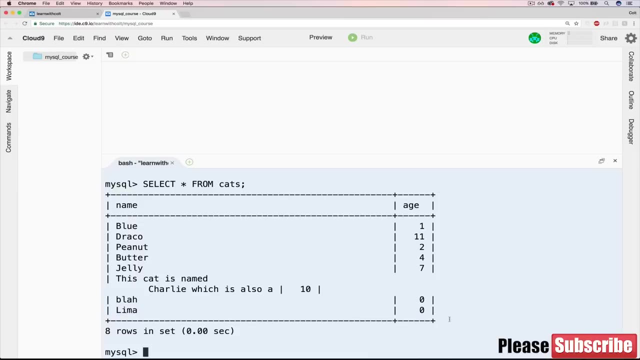 But what do you think is stored inside of age? Any ideas? Well, if we do a select star from cats, we can see we have Lima, Whose age is zero. So in this case, if we screw something up, if we pass in some invalid data or a string instead of number, it will automatically set age to be zero. 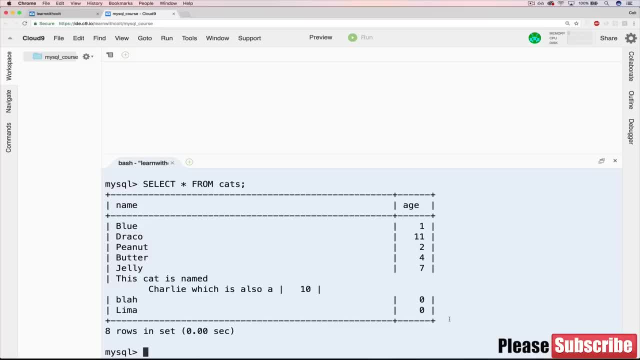 In a little bit we'll see ways of changing that, of changing that default, But for now it's zero. Okay, So that's it for warnings. at this point, Just be aware that if you do see one warning or two warnings or however many warnings after a query, 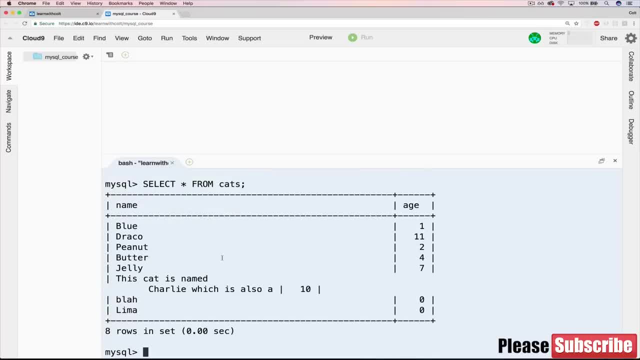 type: show warnings and you'll be able to see your answer. However, actually I forgot to mention this. If we do something invalid, So let's do the same thing, But instead of Lima, I'll call the cat Cusco. 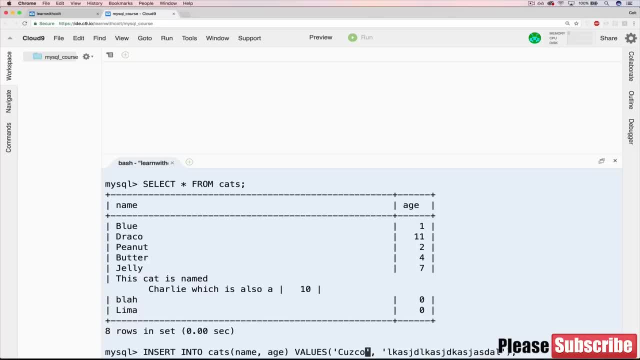 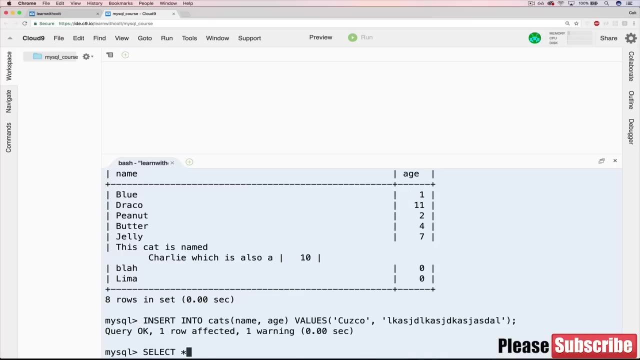 I can't remember if there's a Z in that. I don't know. Well, we'll assume that there is. So Cusco, with this crazy gibberish, should give us a warning. But if I'm wrong, So I do something in between, like select star from cats. 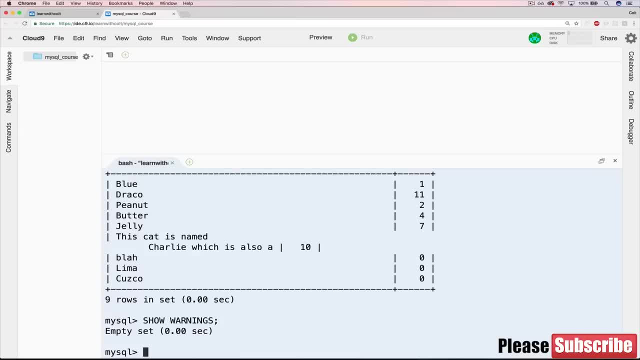 And now I do show warnings, Nothing. Our warning set is empty, So this is just something to be aware of. With that said, when you're creating applications using MySQL, that application, whatever you're using- let's say we're using JavaScript or Ruby- 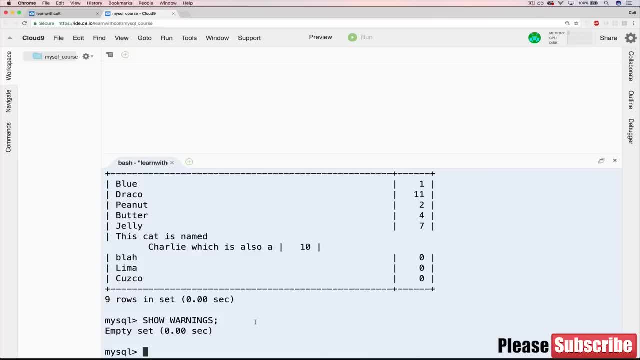 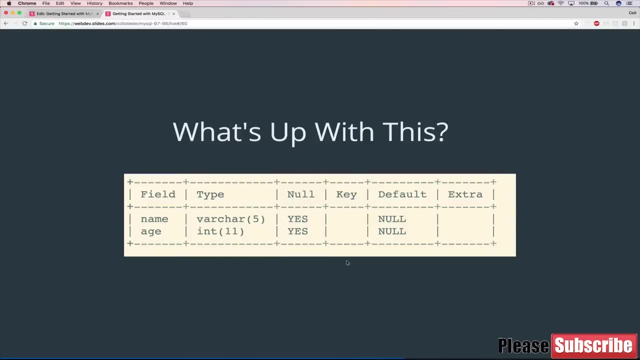 that will have ways of handling these warnings and letting you know. But when you're working in the shell like this, you have to use the show warnings command. All right, That's all there is to warnings In this video. we're going to answer a simple question. 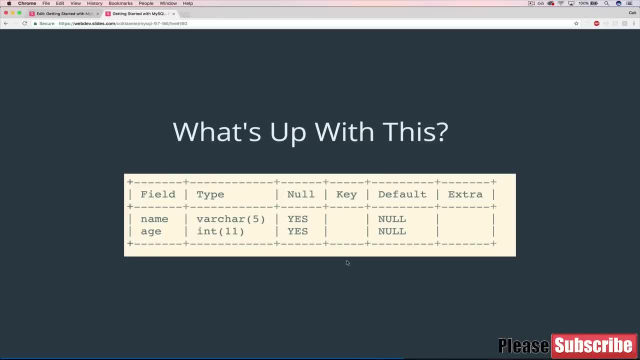 Back when we typed describe table names to describe cats. What's up with this part? What is this null column here in this little table And why is there two yeses for name and age? So this video is all about null, the concept of null. 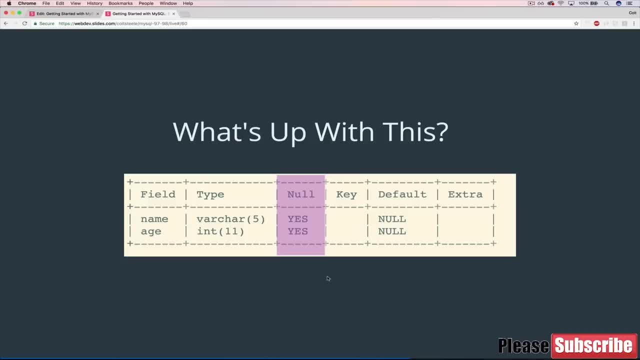 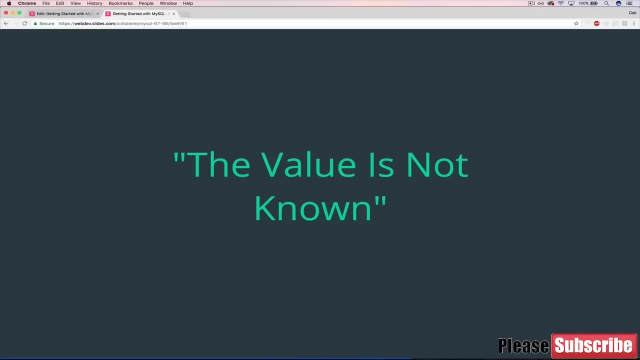 I've been working with null. I'm working with null in SQL. So to start off, let's talk about what null means. Null basically means that the value is unknown. It's SQL's way of saying I don't know what this is, or there is no specified value. 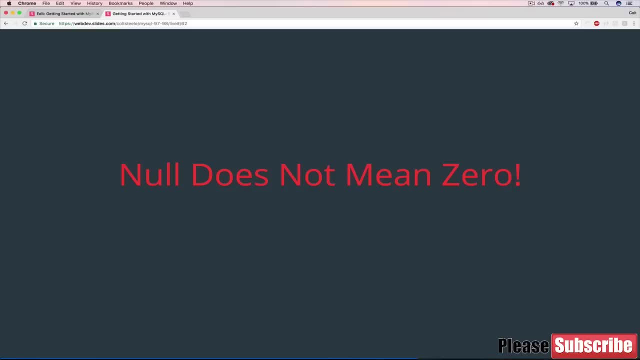 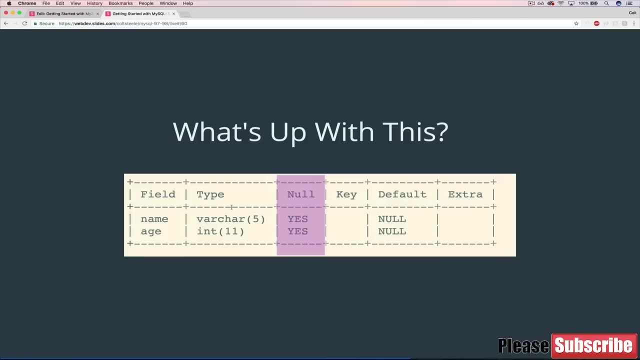 An important note is that it does not mean zero. Some people often think null means zero. It doesn't in this context. So to illustrate the significance of these, having a yes here, it basically means that these are permitted to be null. It's okay if they have an unknown value. 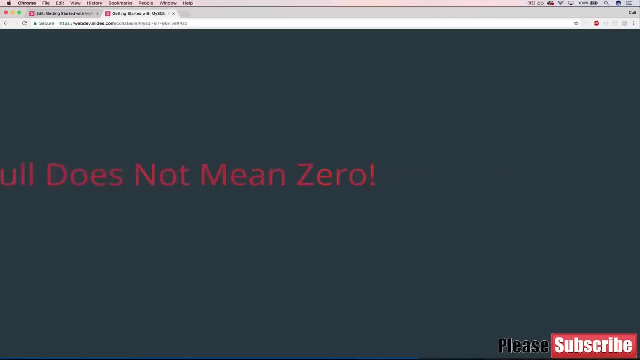 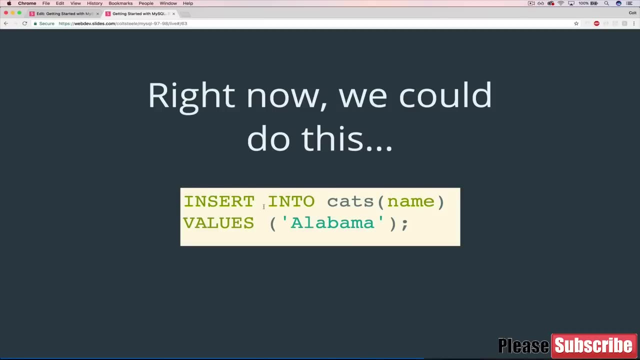 And that happens by default. To illustrate, though, that that is the case, here's a little bit of code. Right now we could run this command. We have a cats table with name and age, But we could do insert into cats and only specify a name. 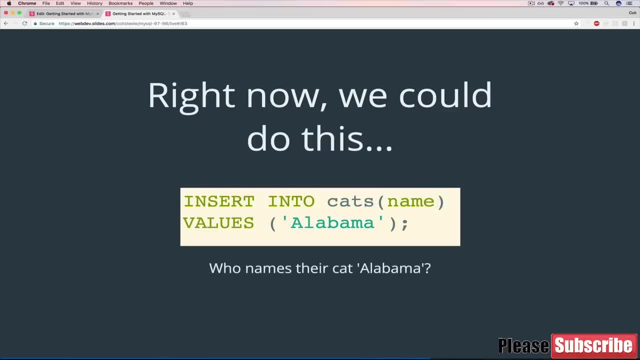 And in this case I used Alabama. I'm not sure who names her cat Alabama, But you could probably say who names her cat, Blue, which is what I named, my cat, So we could run this command. And age has no specified value. 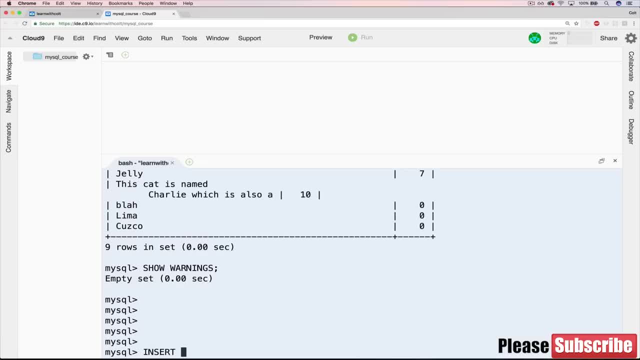 So in fact, let's try it right now. Make some space, Insert into cats name: Oops, Values, What is this siren, Alabama, Just like that. We don't get any warnings or anything saying that name or that age is empty. 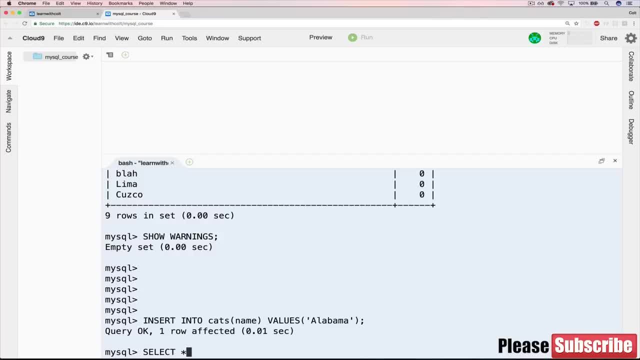 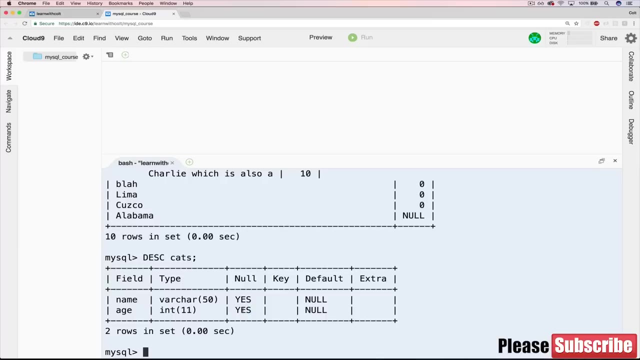 Nothing like that. Now, if we do select star from cats, you'll see that we have a new cat whose name is Alabama, But age is null. And again, that's because we have null as a permitted value. It's technically not a value, but age is allowed to be null. 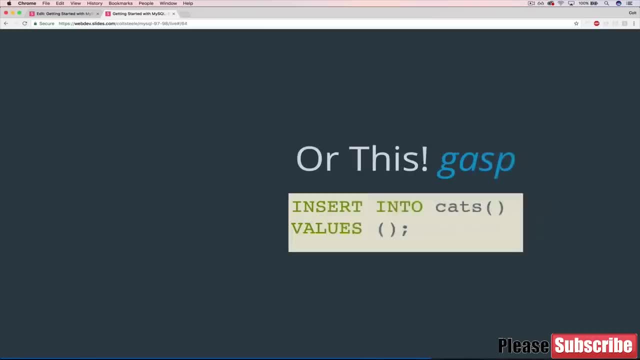 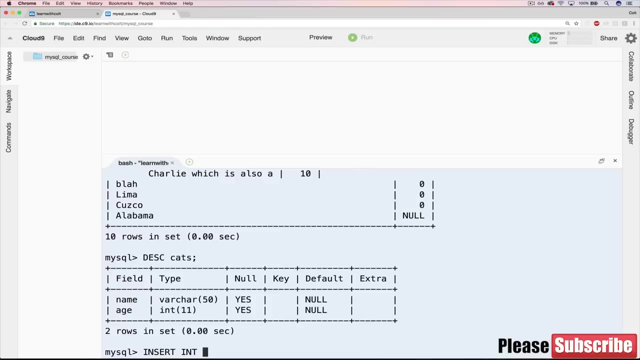 So is name. So I could do the same thing, Or an even more extreme version. I could run this: Insert into cats, nothing Values nothing. And if I did that, take a moment to guess: Insert into cats, nothing Values nothing. 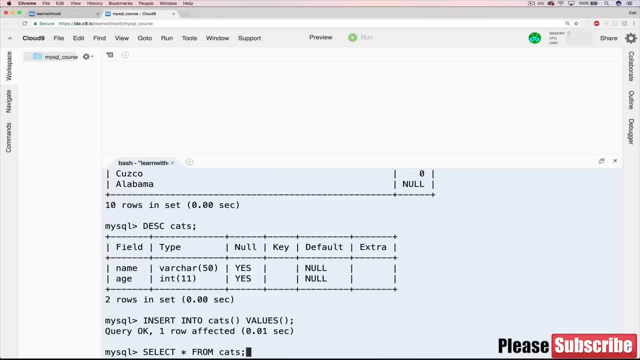 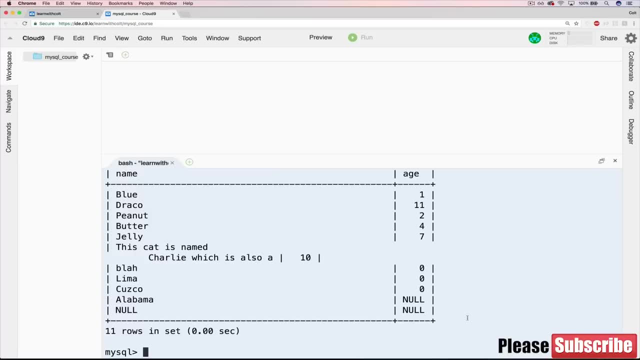 What do you think will happen? Let's do a select star. Now we have cat null or name null, age null. So then the question becomes: how do we prevent that? How do we require that name is not null and that age is not null? 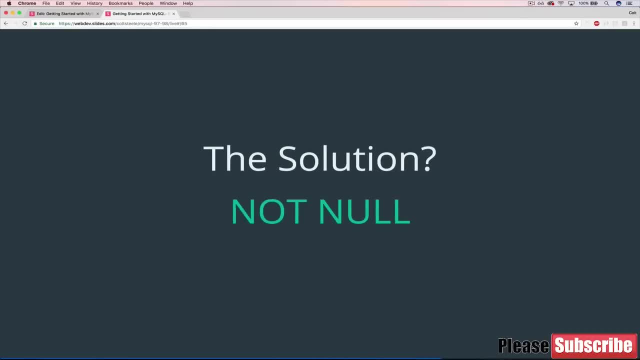 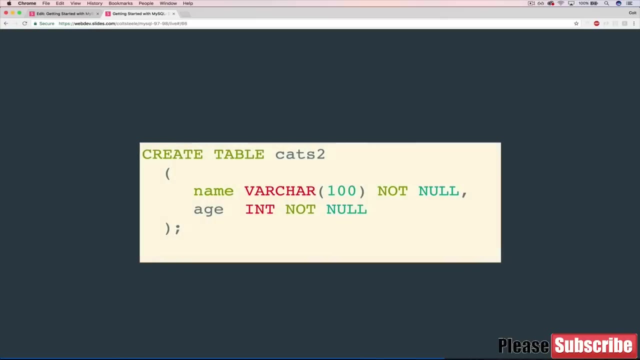 And the answer? And the answer is not null. So what we can do is specify, when we actually define a table, that something, let's say a field like name, is not null, And we use this syntax right here. So here's an example. 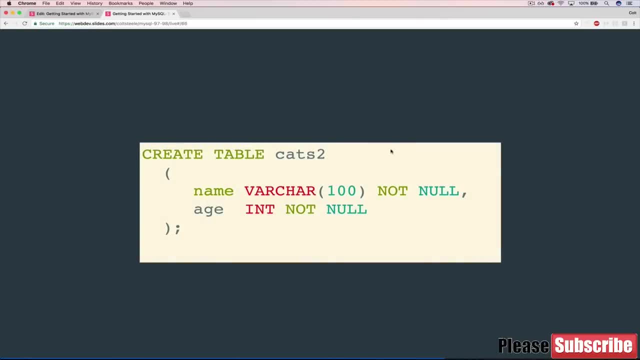 For a cats2 table and I'll be using this convention: cats2, cats3.. So in a cats2 table, our 2.0 version, when we define it, we would say name is varchar. this time I used 100, but the limit doesn't matter really. 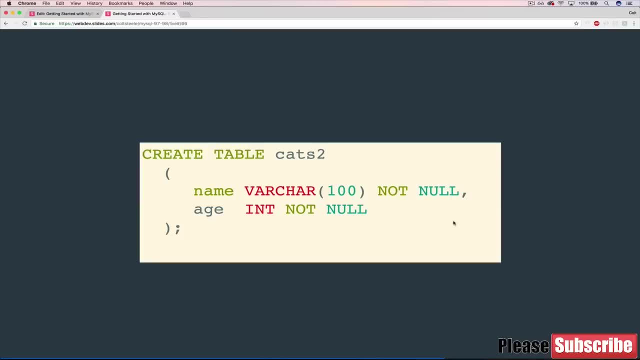 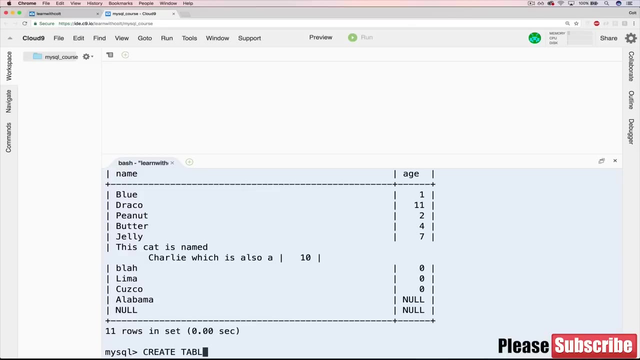 followed by not null. So that means that it will not be permitted to be empty. And then age is also an integer. age is an integer who is also not null. So if we try that right now, I'm going to create a table cats2, and we're going to have 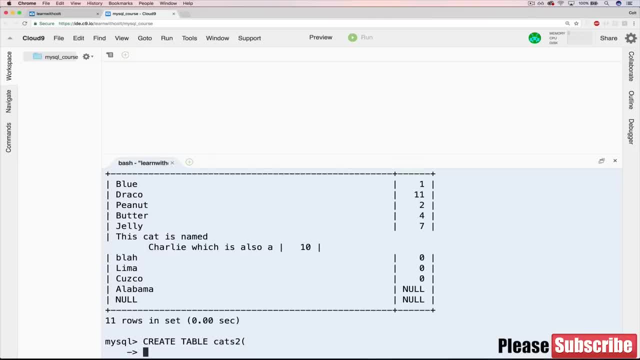 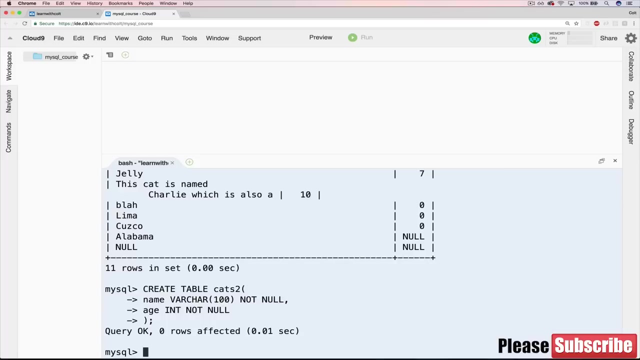 and I'll do this on separate lines. Name is varchar 100,. it's okay, this one. you can have longer names and then we'll have not null followed by age. is an int also not null. We hit enter. 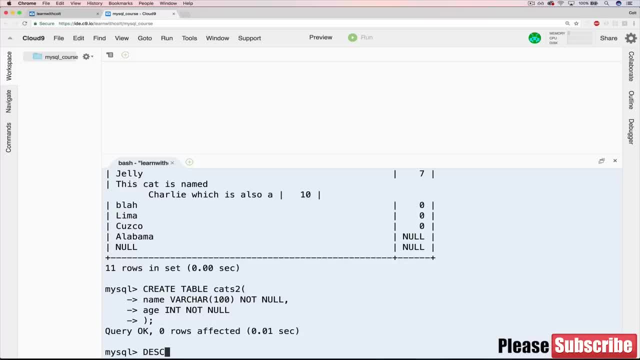 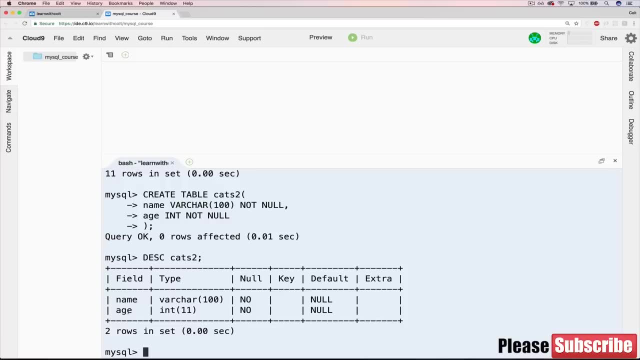 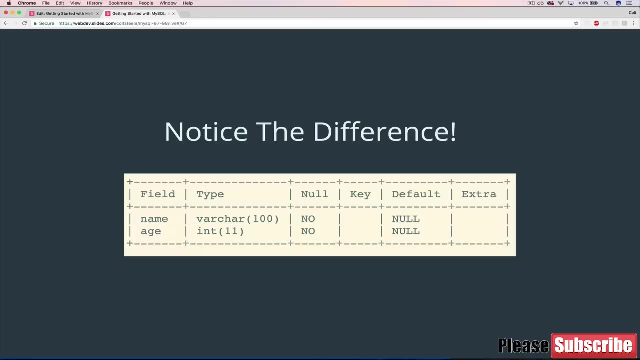 Now let's start off by using describe cats2. cat2.. This time under null, for both fields it says no. So that's one way to tell that these are not allowed to be null. And just to emphasize this, I made a slide. notice the difference here. 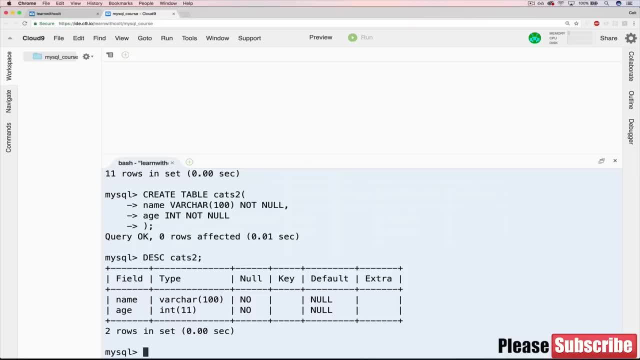 So now let's actually put it to the test. Let's try to insert into cats2, and this time we'll only do name and we'll leave off age, And then we'll have values And name for this one will be Texas, in keeping with the state theme. 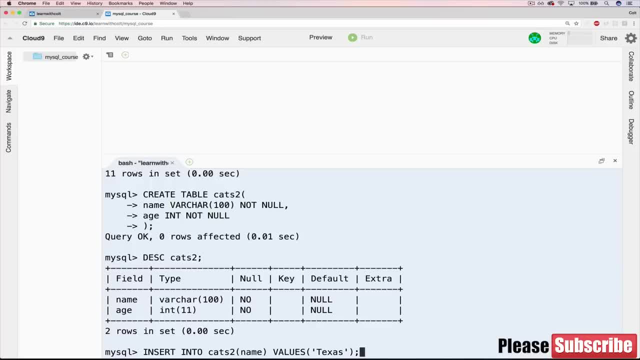 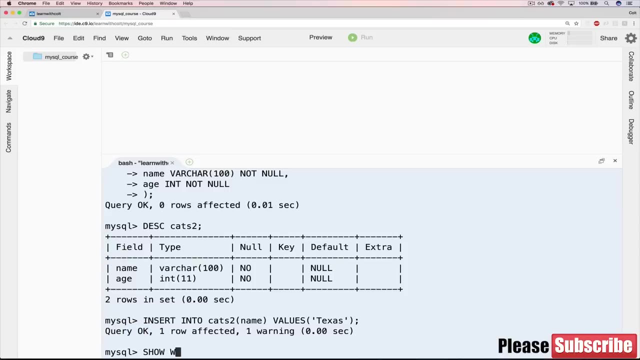 Okay, What do you think will happen? Insert into cats where age is not allowed to be null? but we're not specifying age, So it says query. okay, We didn't get an error message and we got a warning, So let's do show warnings. 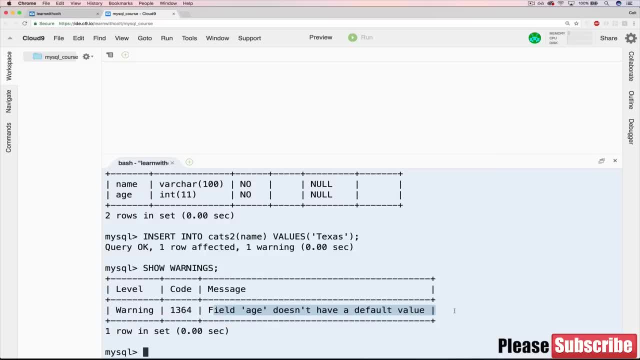 Warning Field: age doesn't have a default value. So what it's telling me is that I left age off, I didn't specify it, So what it was going to do is make it null. But then, oh no, it's not allowed to be null. 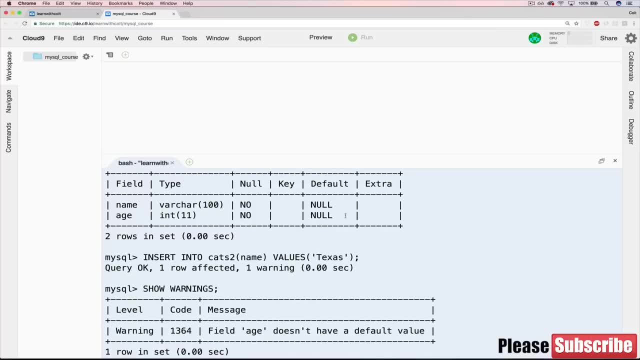 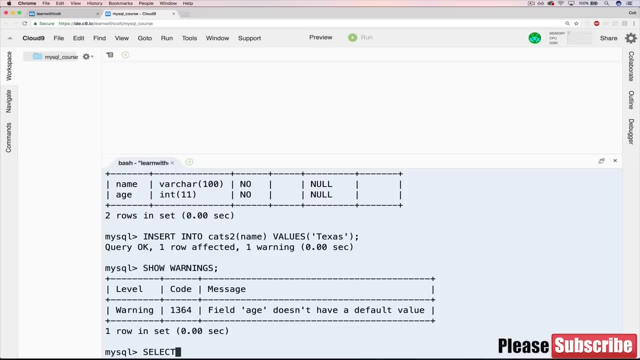 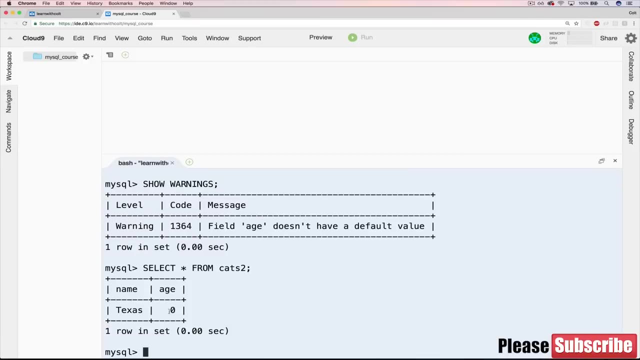 So I need to go find a default value And there's not a default value specified. So if we look, you can probably guess our next video will be on default values. But if we do select star from cats2, you can see it automatically defined zero. 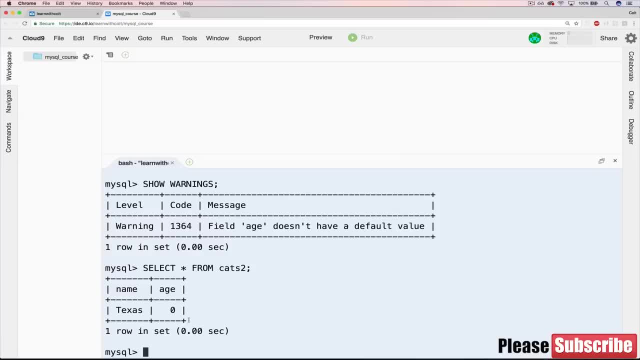 So in the next video we'll talk about why that happened. But the way that int works, if it's not allowed to be null, you don't have a default, it's going to be zero. Now let's try the same thing with insert into cats2.. 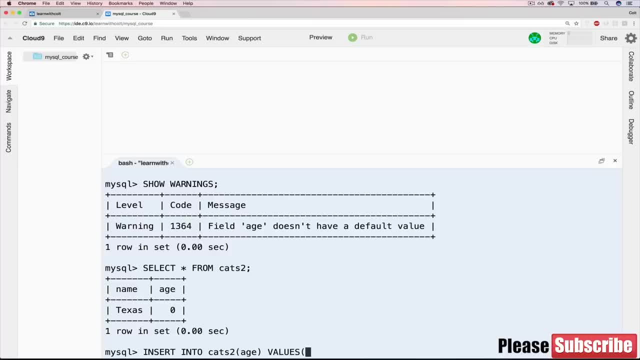 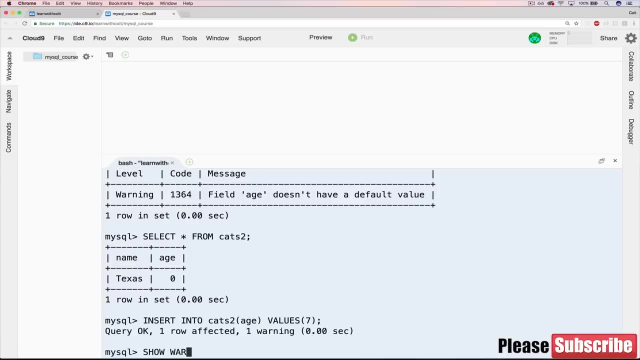 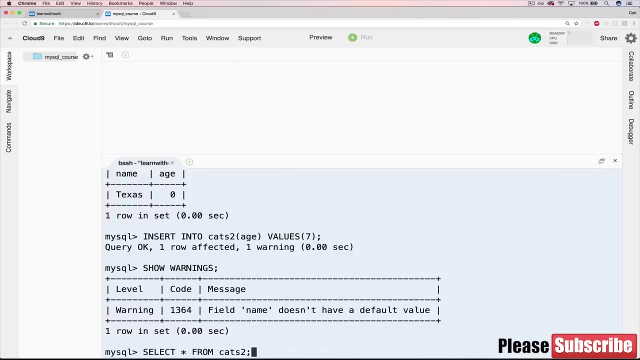 And this time only age is specified, And age will be seven. I get the same query. okay, One warning, Show warnings. This time it says field name doesn't have a default value. Let's do our select star. Notice what we get right here. 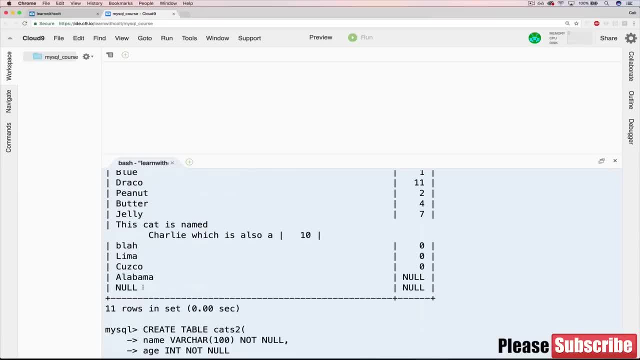 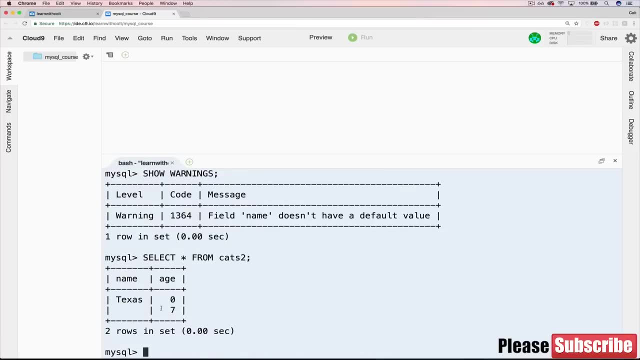 Earlier- see how far back I can go- we had null when we didn't specify a name, when we inserted into cats just regular cats, not cats2.. But now, when I don't specify a name, it doesn't say null. 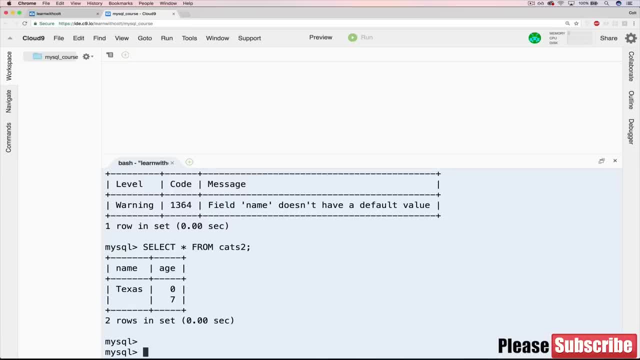 And this is an empty string. So there's a difference. Null means that there is no value at all. We didn't specify Empty string, is just a type of a varchar that just has nothing in it. So you can think of it as this, basically: 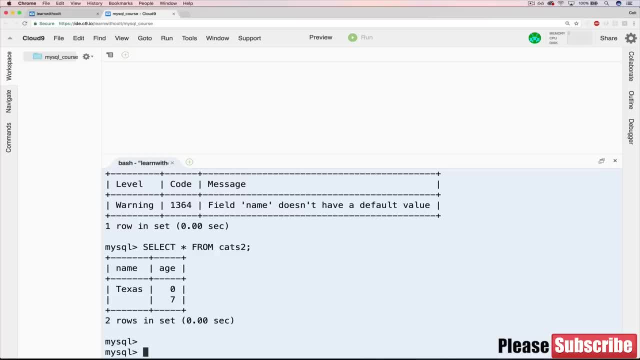 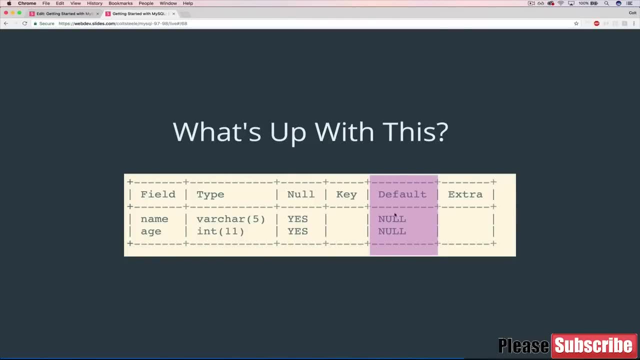 Okay, so next we'll talk about how we specify these default values. Okay, so we're moving on In this video. we're talking about default values. What's up with this part right here? Default. So as we talked about a little bit in the last video, 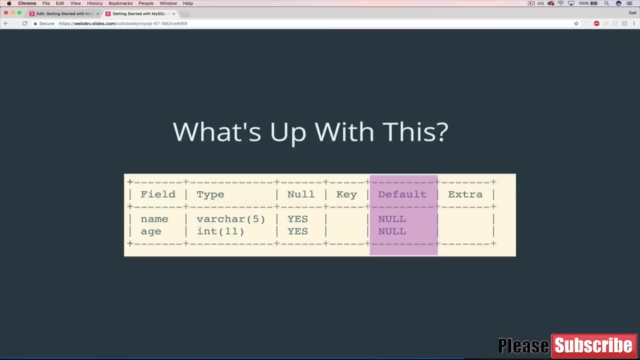 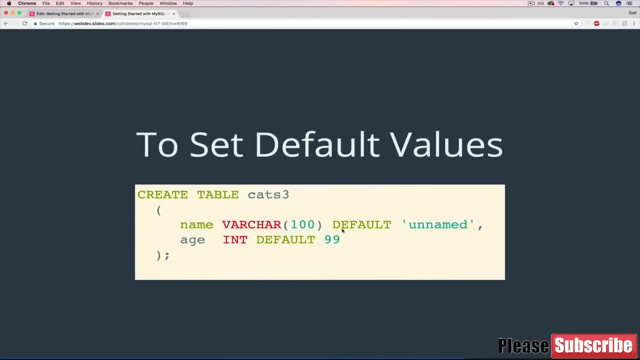 it's helpful to be able to decide or to set default values. So if something is not specified, that there will be a fallback. And here's how we do it: We use default. So you can see both of these when we're defining a table. 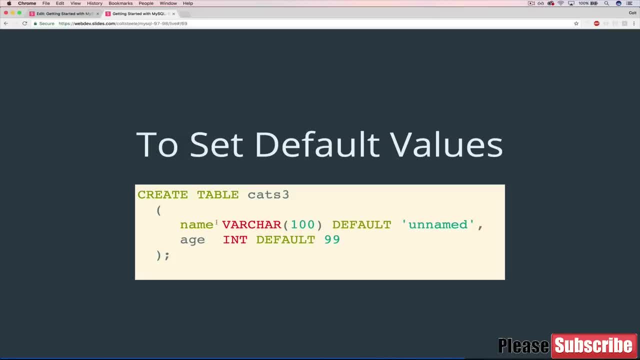 Default and then we specify default. So for name, if you leave off name, I just said okay, we'll call it unnamed Or name to be determined Sometimes. if this is a cat shelter in the real world, sometimes they decide on a name a little bit later. 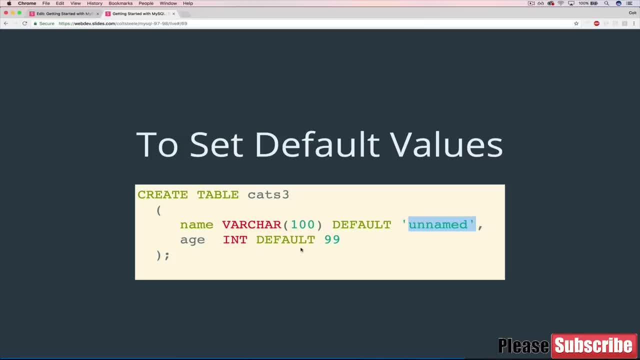 once they figure out the cat's personality, And then for age, if this is more of a silly example, but if we wanted to, if we didn't specify age, we could always set it to be 99.. Not sure why, but for the sake of this exercise, 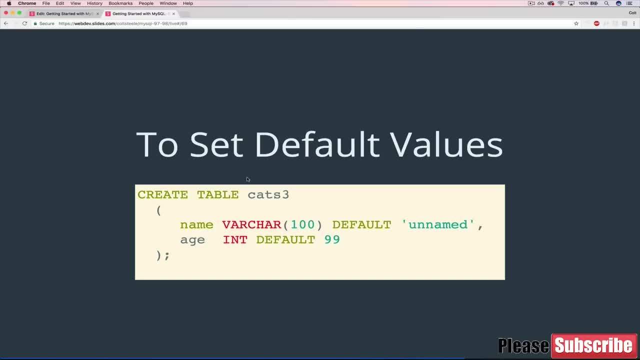 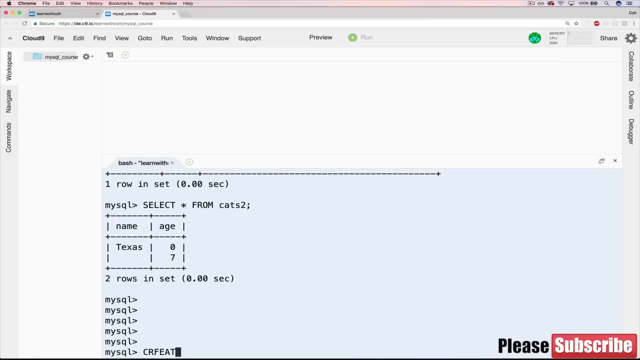 we're going to do that, So let's give it a shot. Remaking a new cat's table cat's three. Okay, here we go. So create table cat's three And I'll do a new line here And we will have name. 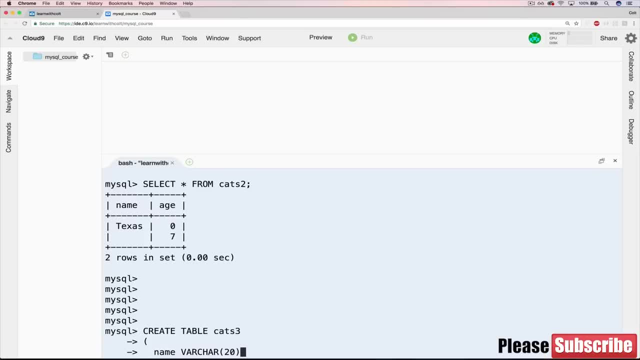 var car, Let's do 20,, even though my slides say 100.. It's okay Default and our default will be: let's see no name provided. How about that? It's important that whatever you put here matches this data type. 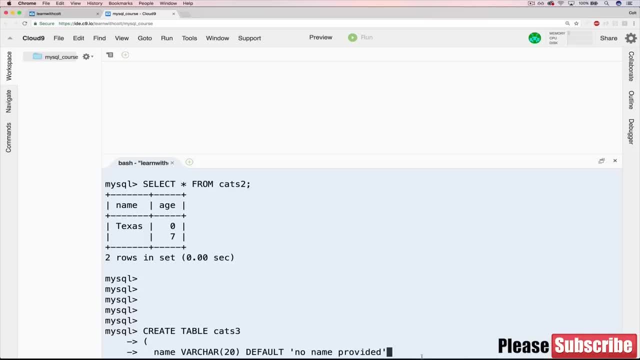 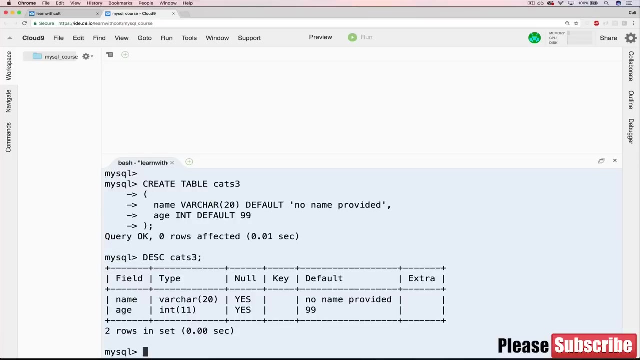 So we couldn't say the default is the number 100. And then we'll have our comma: Age and age is an int. Default should be 99.. Perfect, Close that. Now, if we do our describe cats three, here we go. 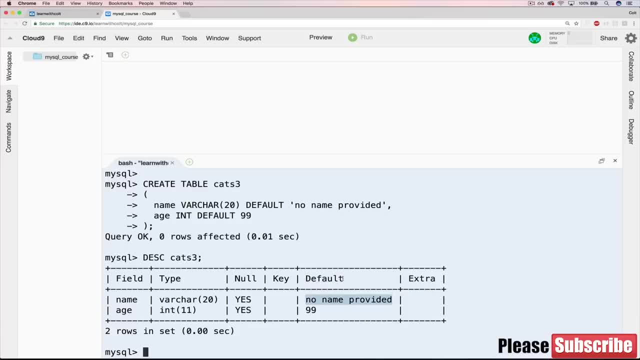 So we have default: no name provided, default 99 for age- Awesome, Okay. so now let's give it a shot. Let's do insert into cats three And I'll do age only and no name, And age will be. 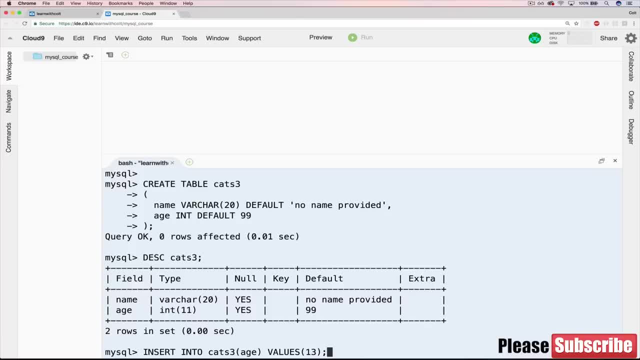 let's do 13.. Just like that. What do you think will happen? I'm going to insert a new cat into cats three, which is right here. Only providing age And name has a default value of no name provided. Okay, I did it. 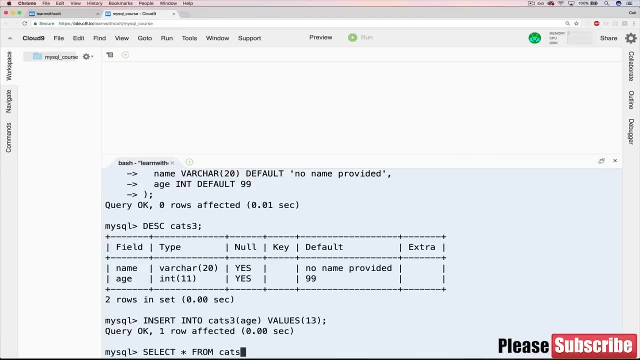 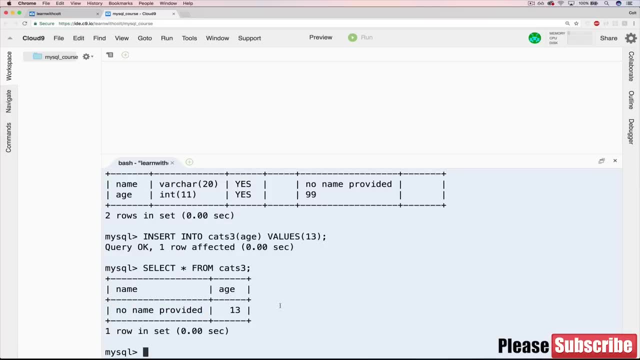 Now let's look: Select star from cats three And I get no name provided. Perfect, So we have a default value. That's working great. We could do the same thing for age. Feel free to skip this if you feel like you know exactly what's going to happen. 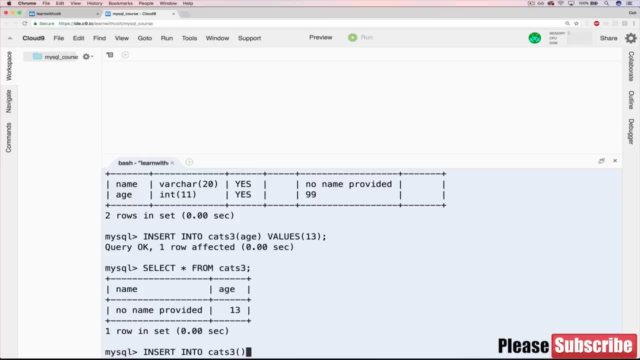 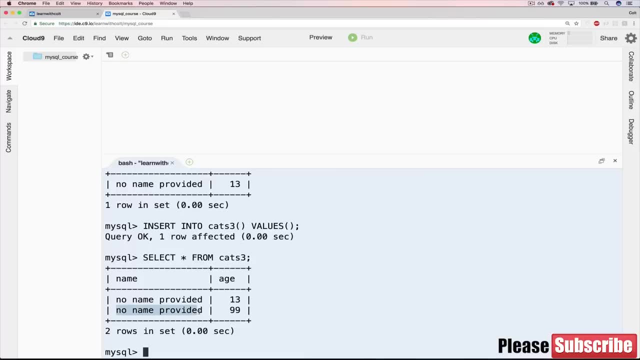 I'll leave. let's leave both off this time. Insert into cats three values. Now when we select, we have another unnamed cat, This time who is 99 years old by default. So the next thing that I want to talk about: 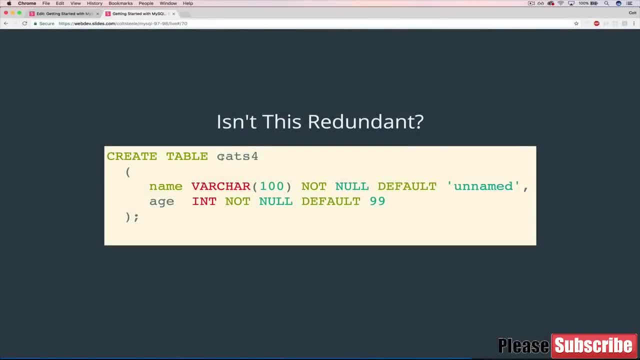 here's another version of creating a table for cats four, this time And I combined not null alongside default. Otherwise it's the same. So we have name: varchar: default is unnamed. age: int: default is 99. But I added in not null. 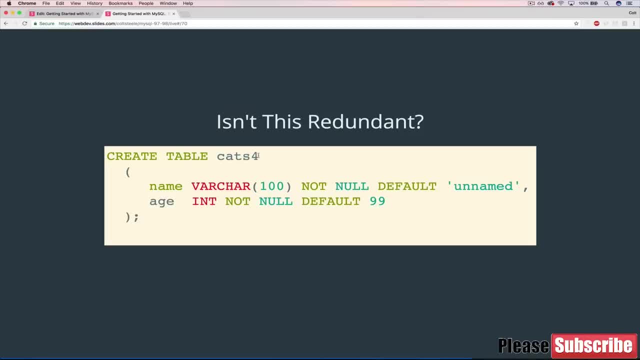 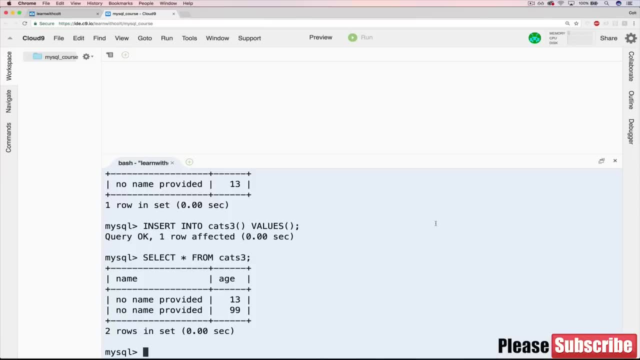 And, as I wrote here, you might be thinking: is this redundant? Because if we have a default value, it's already saying it won't be null. If we go back and we look at cats, regular cats, if we do an insert into cats, 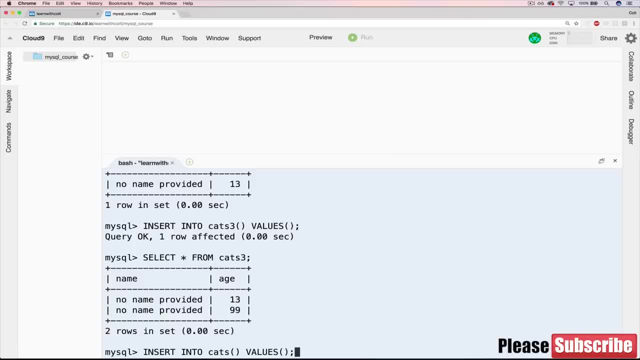 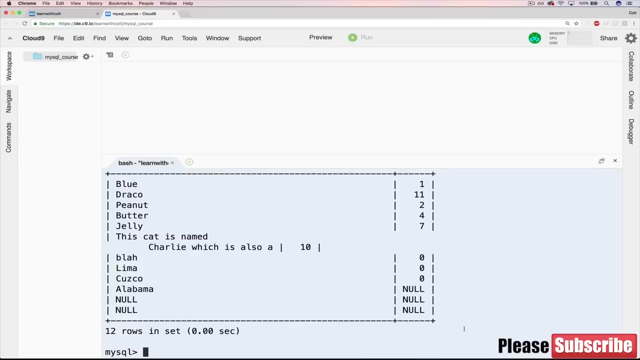 just like this, And if you can remember, all the way back to cats, we have no default provided. And I do select star from cats. We get no, no, there's no default values. And then when we have our cats, three: 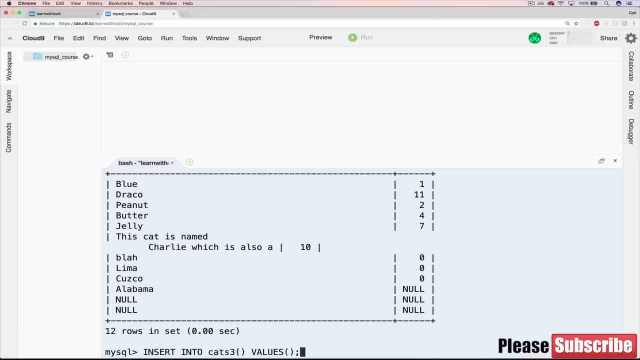 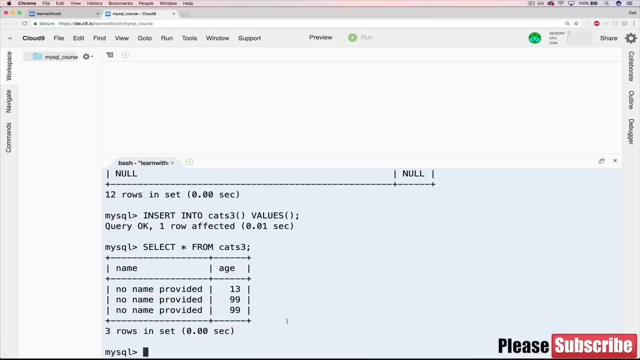 when I insert something like this right here, insert into cats three, it's totally empty. We have those defaults. So when I select star oops from cats three, we get no name provided 99. So why would we want to add not null? 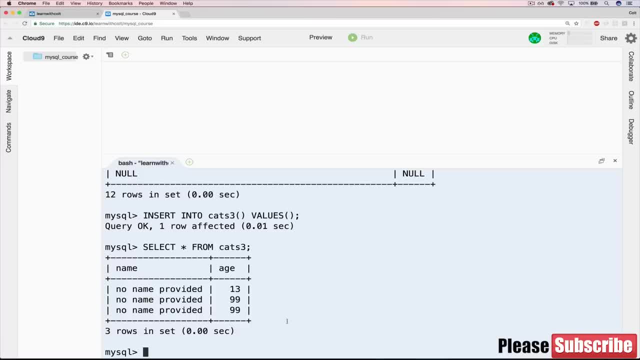 And the answer is that we could still manually set something to be null. So if I did that here, let's do inserts into cats three And I'll do name and age, name and age values And I will say: there's no name. 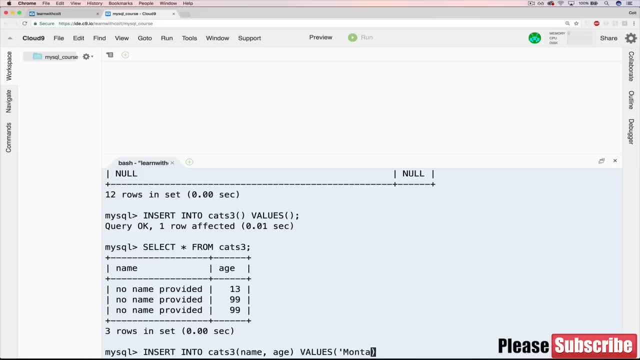 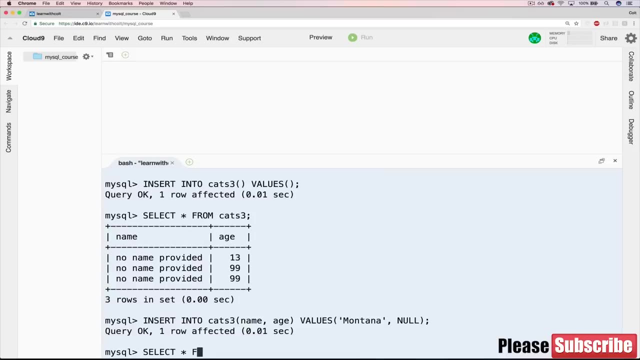 All right, let's say name is what's? another state in Montana- It's not too bad for a cat's name, Great state, by the way- And we'll leave age as null, explicitly null, just like that. Let's do select star from cats three. 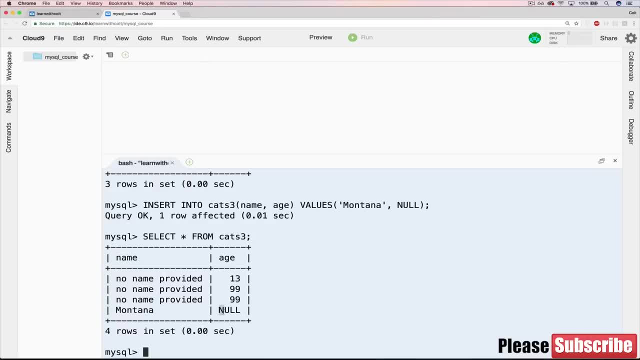 And you can see that there was nothing stopping us from setting age to be null. All that we have is a default value. If you don't specify something, it will be 99, but you're allowed to say no. I'm allowed to say this is explicitly an empty value. 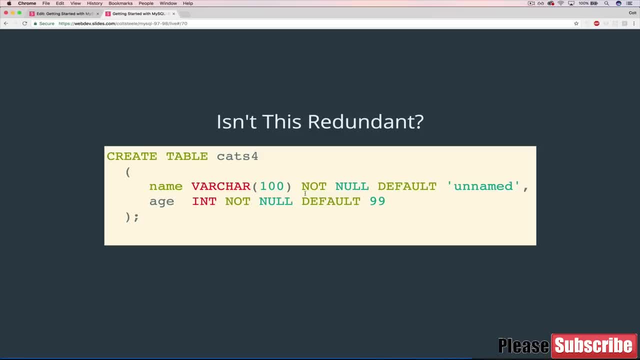 Okay, So that's where this comes in: Name varchar, not null and a default, And I won't make you sit through me typing that whole thing, So I'll just copy it. But to walk through it again, same thing here. 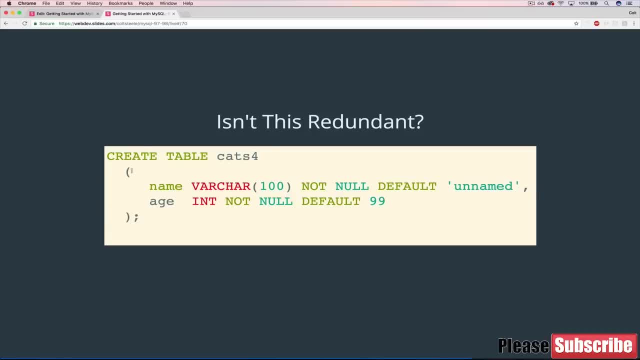 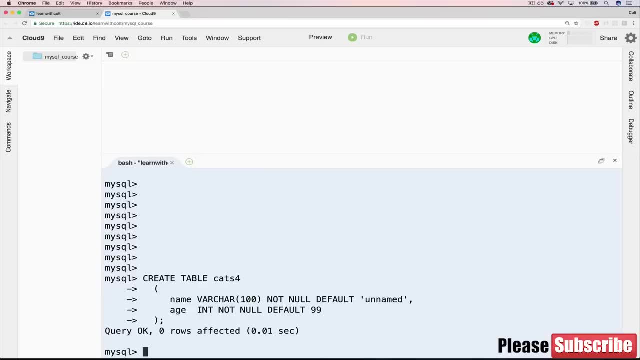 Same with the default. We just added not null and not null. So let's go ahead, paste this in: This is cats four This time. if I do describe cats four, we now have null is no on both and we have a default on both. 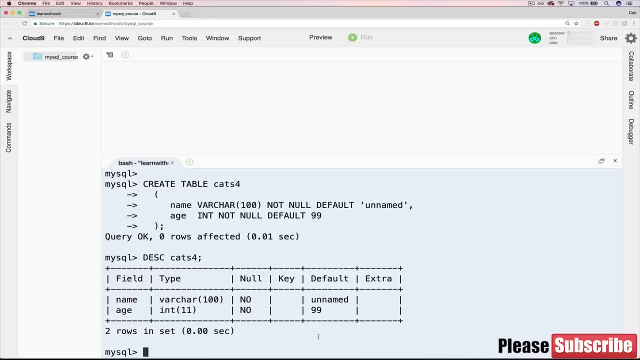 So we're almost there. I know it's been a little bit of a long video. Let's do a insert into cats four And we will specify name and then age, And this time, if I do values, oops, and I say name is. 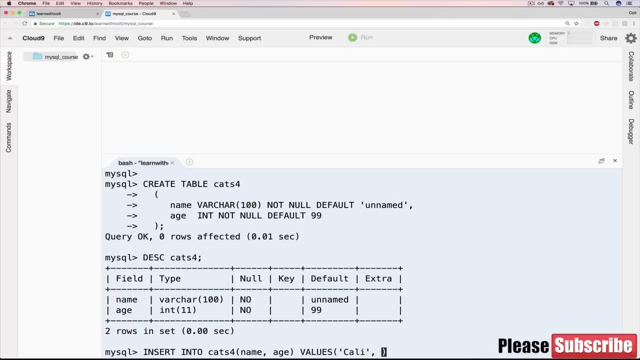 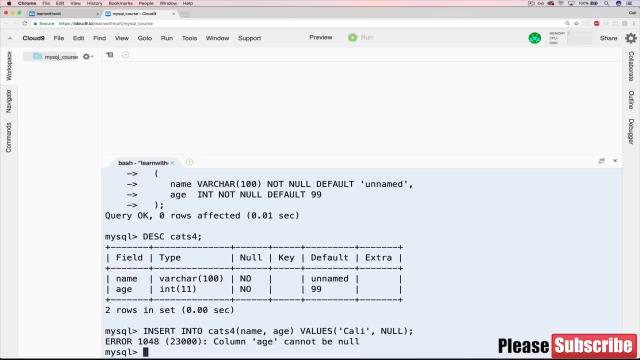 what's in it. Let's do Cali Fine Sort of a state name And age is null. If I do this this time we get an error. So not just a warning, but an error saying it cannot be null. 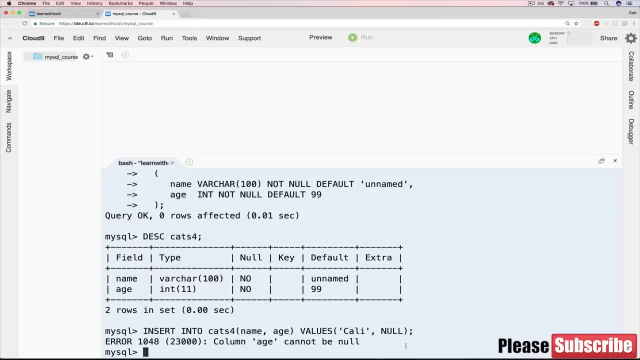 And that's what not null specifies. So important to note that You'll use not null pretty often. It's a way of basically requiring that something has a value, But also saying that it's not allowed to be null itself, which I also included as a slide here. 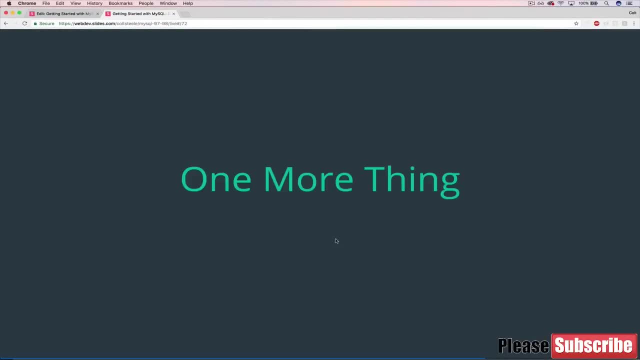 In cat three, we can manually insert something as null. Okay, As you can see, the slide says we have one more thing, And that is true. We have one more thing to cover here before we do our final exercise in this section. 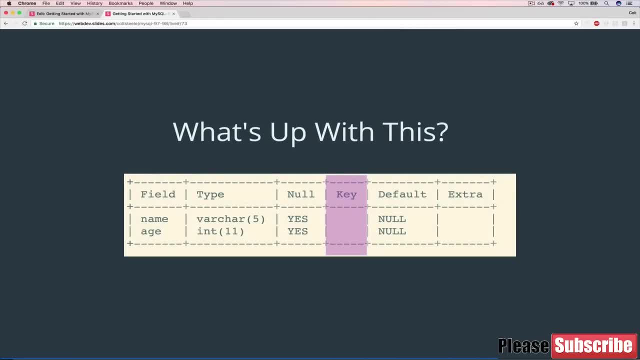 So, in keeping with this pattern, what's up with this? This key column here And it's empty. There's nothing for name or age. What does this mean? So, to dive into this- and this is actually something we are going to come back to- 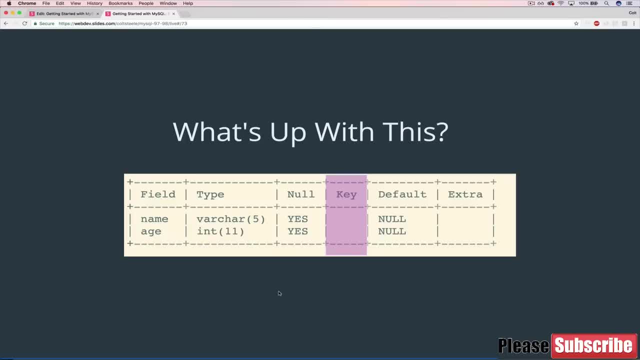 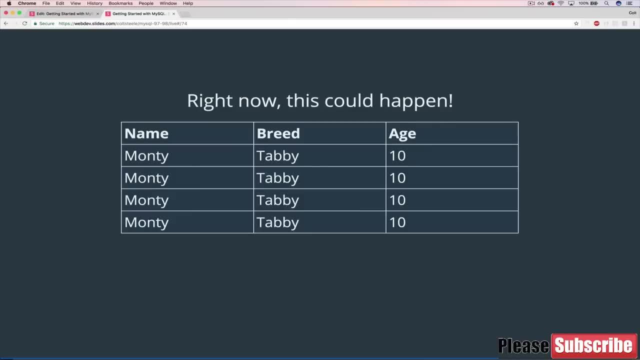 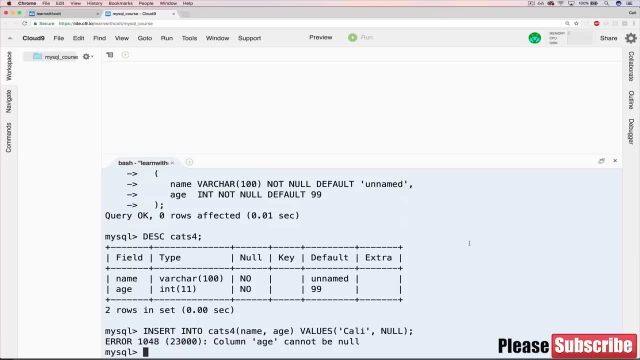 And we've already seen this. but just to prove that to you, if I just work with cats, let's do select star from cats, And this is true about any of the cats tables we have. You can actually already see we have two cats that are identical. 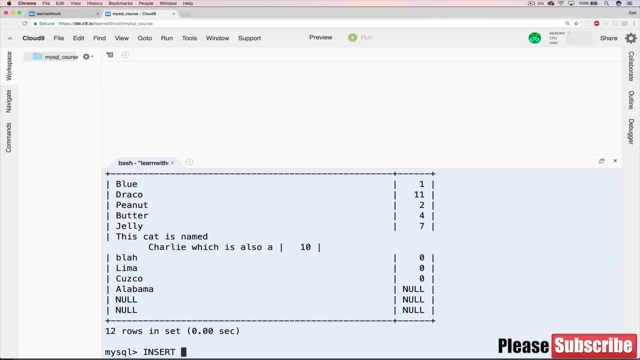 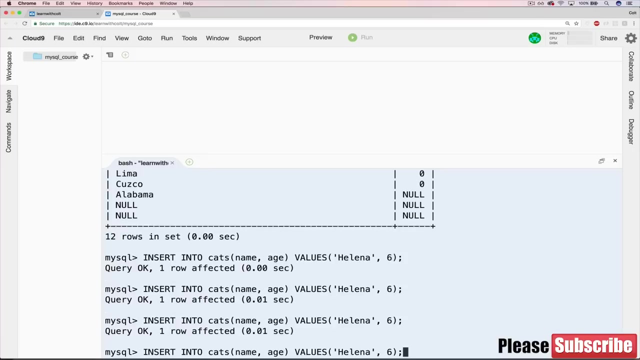 Null and null. But I could also do something like insert into cats Name age values, And this one will be called Helena, And Helena will be 6. Or Helena, however you say it. We can do this, And we can do it as many times as we want. 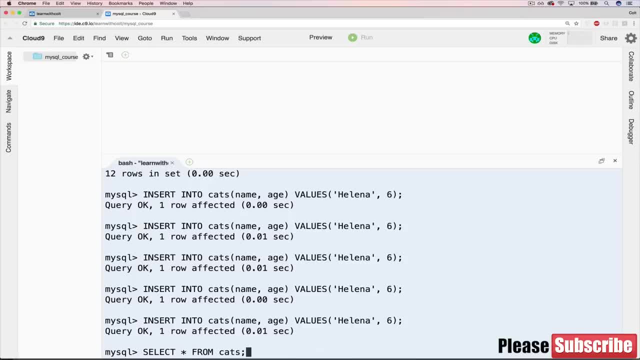 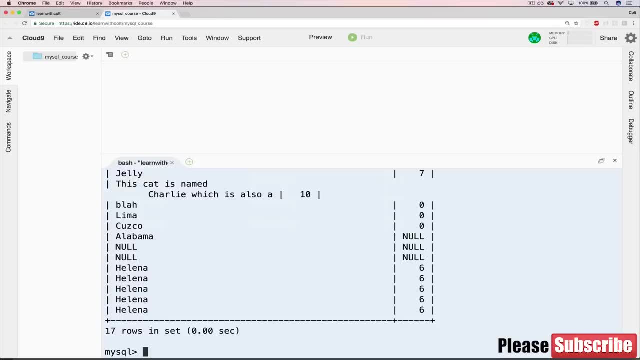 And there's going to be identical data in there. As you can see, we have five identical cats, So why should you care? Why is this really a problem? And there's a couple reasons, But it comes down to the fact that we want all of our data to be uniquely identifiable. 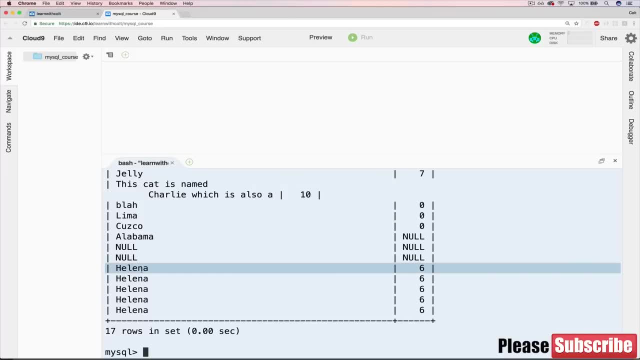 Even if it looks the same, like it does in this case, we assume that these are separate cats. If they are in fact one cat, then this is just in error. We don't want to have this many entries, But imagine we actually have five cats named Helena, with an age of 6.. 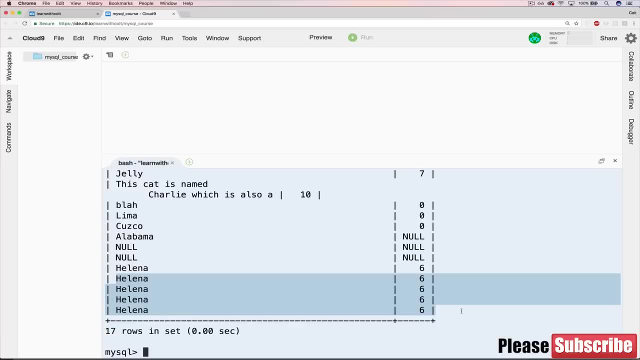 They are unique and individual And we want to be able to keep track of them And right now we can't. There is no way to uniquely refer to this. So in a case like here, where we have Alabama, who is null, age null, 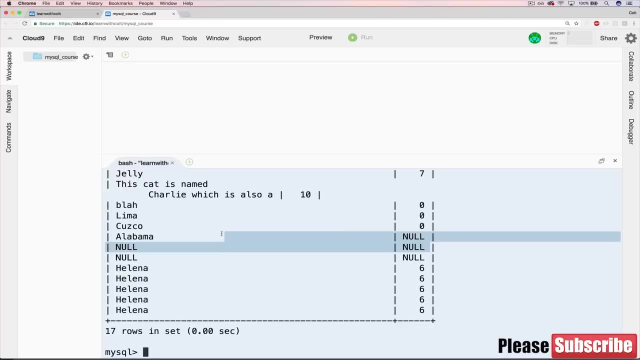 and then we have Null, who is age null. there's a way of telling these apart, Even though they both have an age of null. I could tell SQL, and we don't know how to do this yet. but I could say: give me a cat whose age is null and whose name is Alabama. 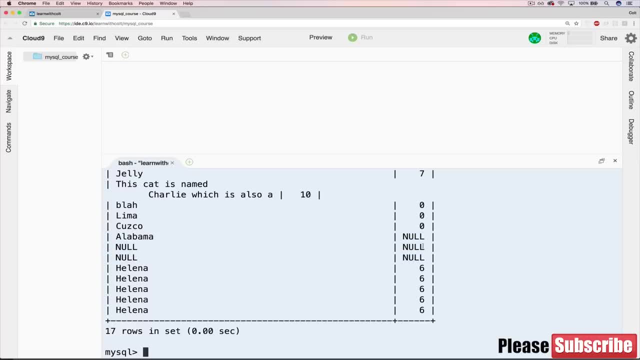 And that can get me this, But there's no way for me to get this cat and separate it from this cat, or this one and separate it from this one, And that's really a useful and important thing And it's actually a really fundamental part of working with databases. 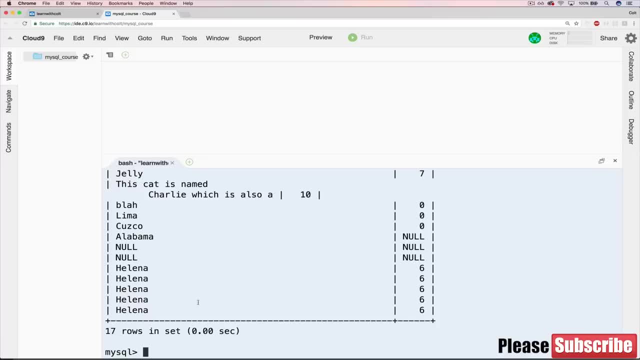 It's having things be identifiable. When you're signing up for an account on, let's say, Twitter and you're trying to make a username, there's a reason that you can't just make the same username that already exists. I wish that I could just go and make my username Colt. 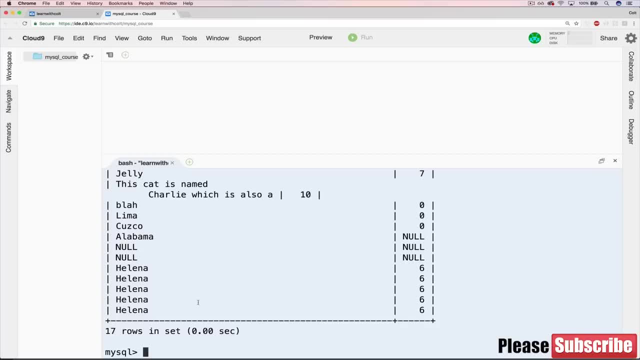 but somebody already has that. And it's not just about keeping it simple and not being confusing for users, because obviously it would be confusing if there was one Colt and then another Colt and they're both tweeting. how do you know who is who? 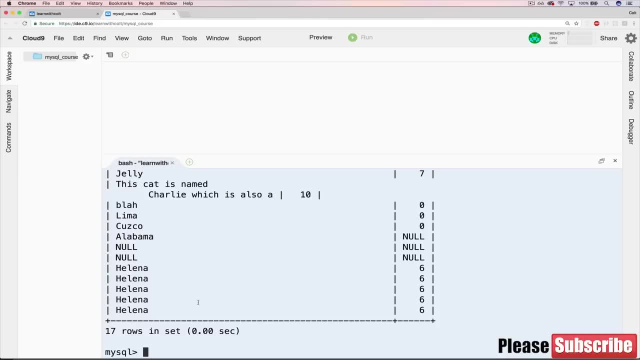 But actually in the code that's hugely problematic because there's things like when I log in I type my username and it's going to go to the database and try and find a user with username Colt and then it's going to match my password. 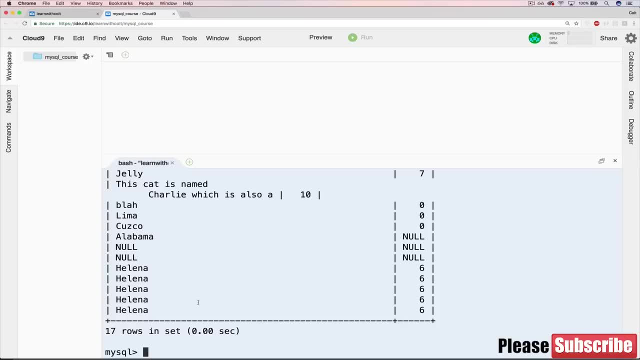 But if there's two users with username Colt, then what does it do? So in that case you're not allowed to have separate usernames, But there are times when we have data that looks the same, Like hypothetically we could have two cats named Helena. 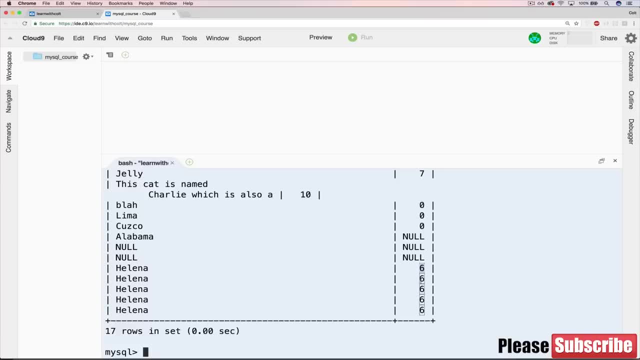 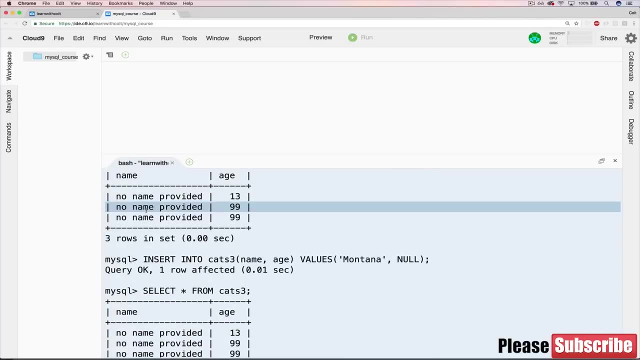 age six, Or maybe a better example, we could have a couple of cats if we go back here where we have no name, provided They're unnamed, but they're unique, different cats. How do we know? And the easiest way? 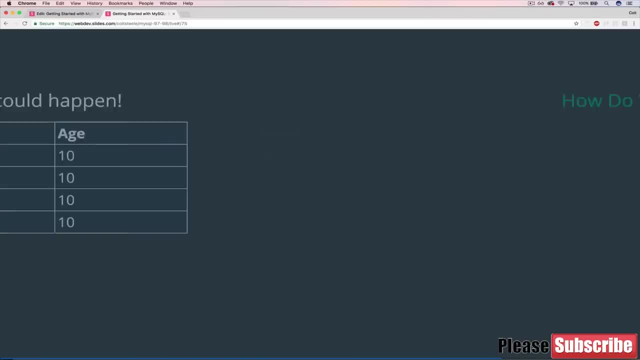 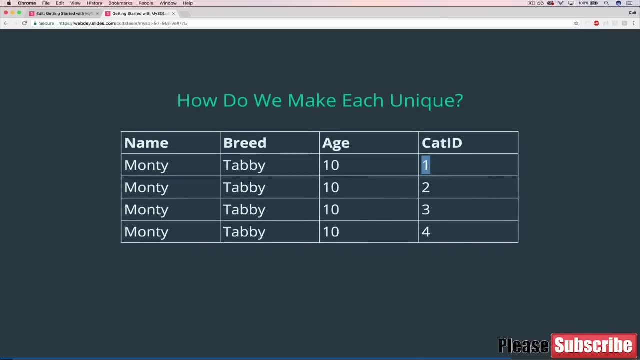 and what we'll do, and what pretty much everyone does, is assign an ID, So a unique identifier. So you can see, here I added a new field, cat ID, and every cat is given one of these IDs. So now, 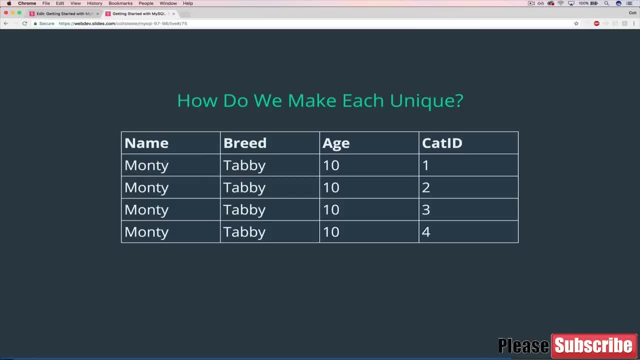 rather than saying I want to select Monty from this database and getting all of these, I can say I want the cat with ID one or ID three and they are uniquely identifiable. All right, So there's a precise term for this. 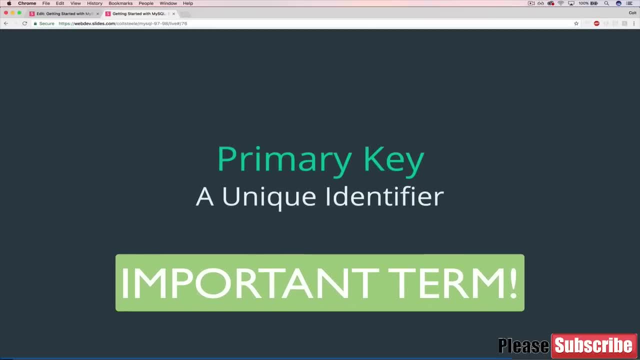 primary key. So a primary key just refers to something that is a unique identifier on a row. It's a way of identifying something and you know that it will be unique. Just a heads up: we will see another type of key later on. 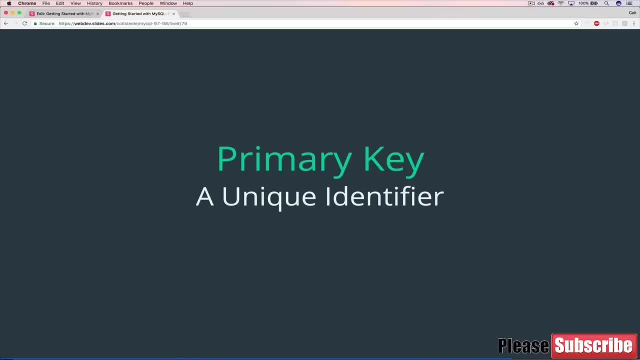 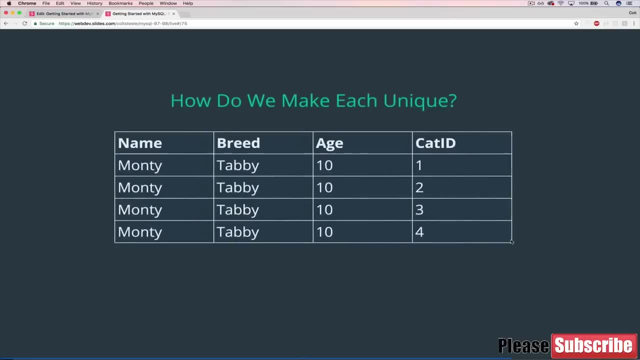 called foreign key. Those are both keys, Don't worry about it. but primary key just means that whatever field we assign, whatever we make the primary key- so in this case we would make cat ID a primary key means that it has to be unique. 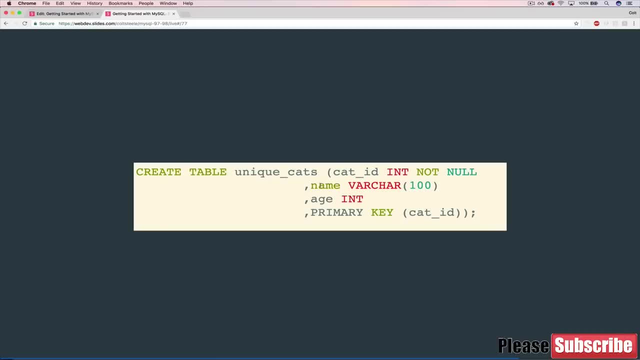 So let's see how we actually assign one. So I'm creating a new table here and I know it's a little bit longer than what we've seen, but a lot of it is very, very similar. So we have unique cats. 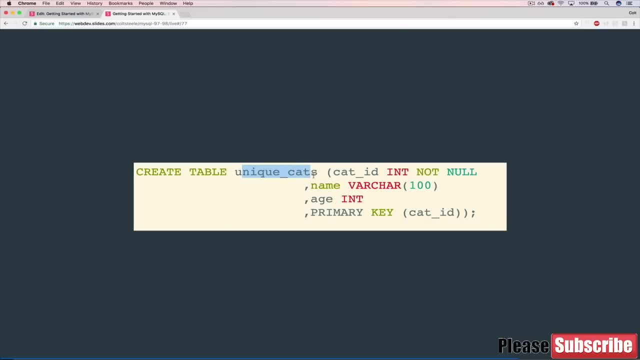 it's just the name of the table, just to. I got tired of cats one, two, three, four, So unique cats. we have name and age, but we also have cat ID now. So cat ID is an integer and we can't have cat ID be null. 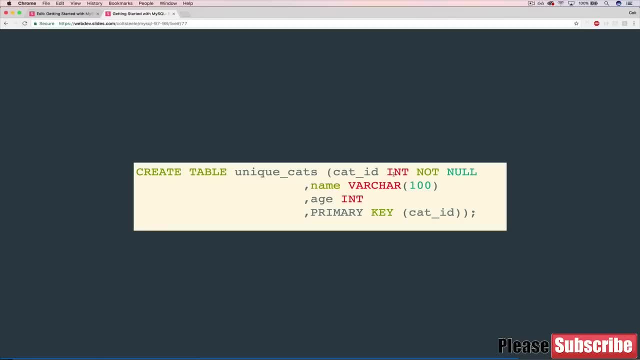 We definitely want there to be something there. and then this is the new and important piece. This is just another field. This isn't technically new, conceptually, but this is primary key. And then we give it the name of a field, So we want the cat ID to be unique. 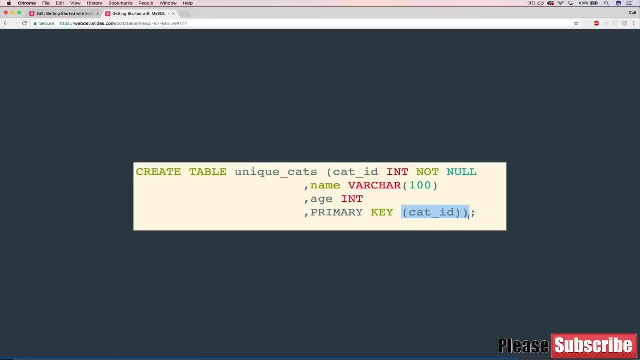 We want it to be the unique identifier, So we just pass it in here: cat ID. So let's try this out. I'm just going to copy it over, just to save you time, So you don't have to watch me type the whole thing. 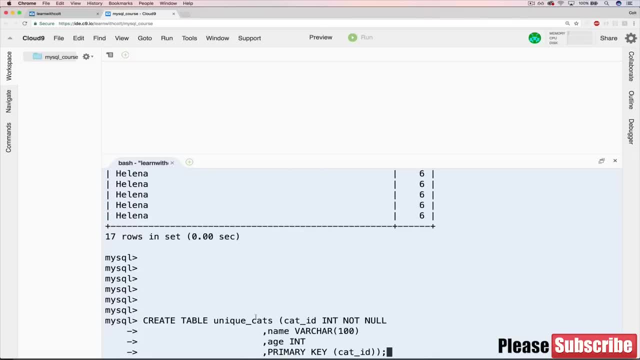 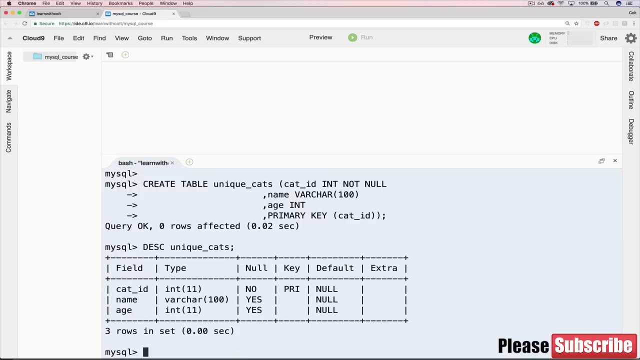 Here we go: Create table, unique cats, cat ID, name, age And, by the way, that cat ID you talked about earlier is a primary key. All right, So now let's do describe unique cats And you'll see a couple of things. 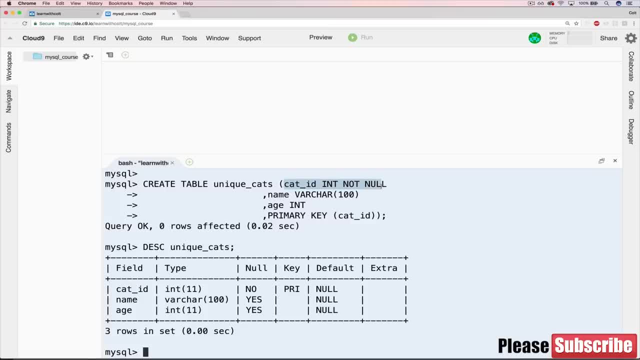 We have cat ID now because we had this line here. but we also, under this key column, we have primary or pry, But it means primary key. So cat ID is a primary key. So how do we know? Well, let's insert into cats or unique cats. 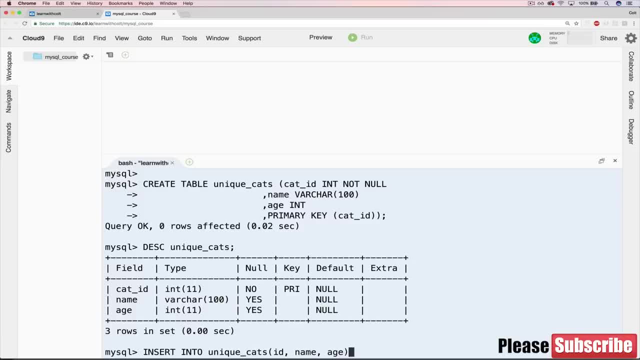 We'll do ID, name and age, just like that, And then we'll do values And we'll start off with an ID of one: Name will be Fred And age will be one, And let's do two, Fine, 23.. 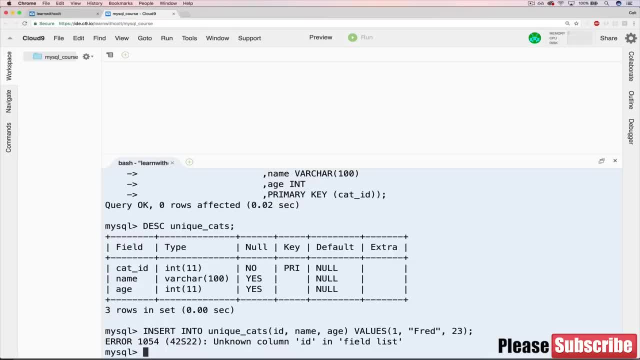 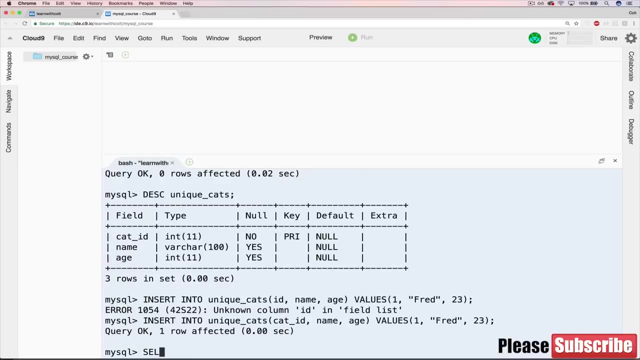 Accept the typo. Okay, Hit enter. Oh, we have a problem. I just referred to ID. It should be cat ID. Silly mistake. So let's fix that Cat ID. Okay. So now just double check our work from unique cats. 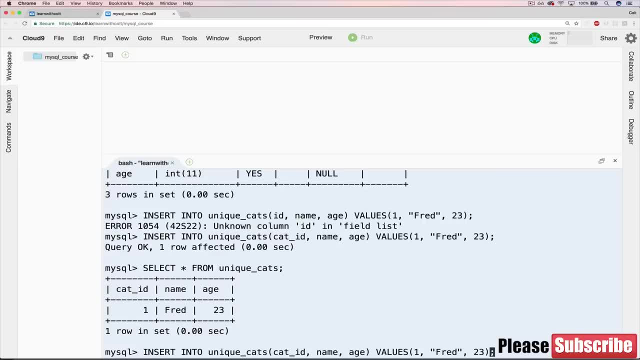 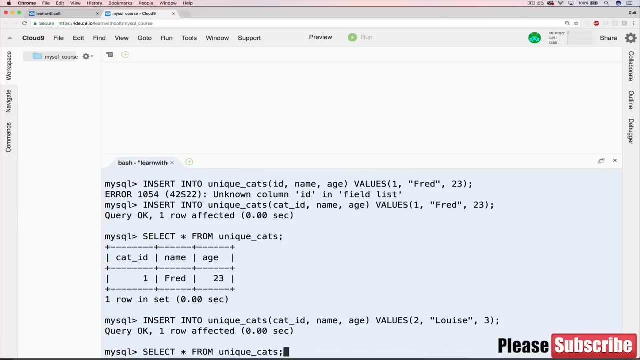 Cat ID is one. All right, Let's do the same thing. Change this to two, And instead of Fred, let's have Louise, who is two. Three, We hit enter Same thing. I think you get where I'm going here. 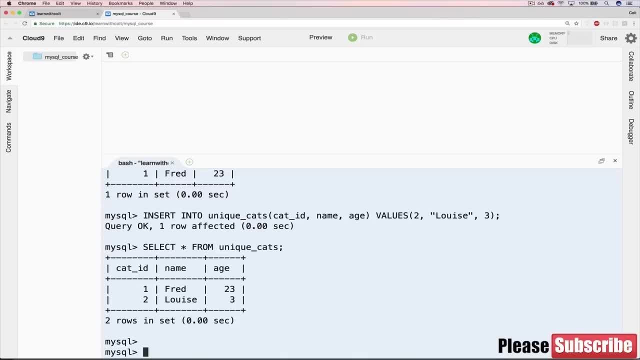 We can keep doing this. However, and this is where the primary key part comes in- I can now say: insert into unique cats cat ID name, age. What if I tried to make another one with ID one, And this one is called James? 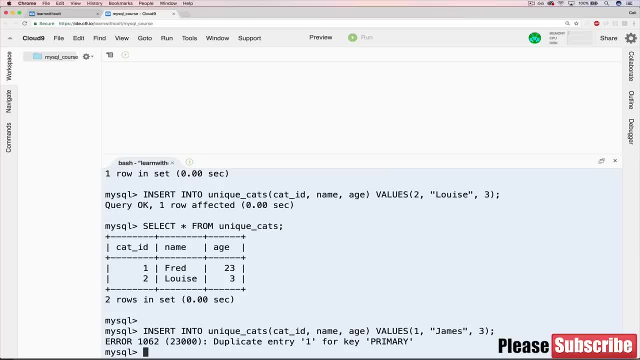 Just like that I get a new error: Duplicate entry, one for key primary. So this is saying: wait a second, You said it's a primary key. I cannot have a duplicate entry. You cannot have something. The whole point is that ID is supposed to be uniquely identifiable. 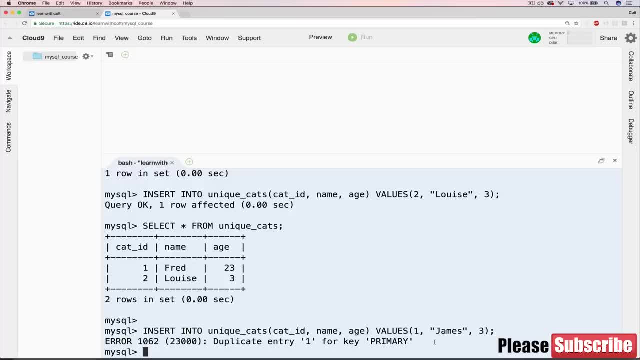 Well, that's a problem, So it doesn't add it to the database. So that's really, really important. And IDs are not the only thing. you can make Primary keys. I gave that example of username, which is something we'll come back to later. 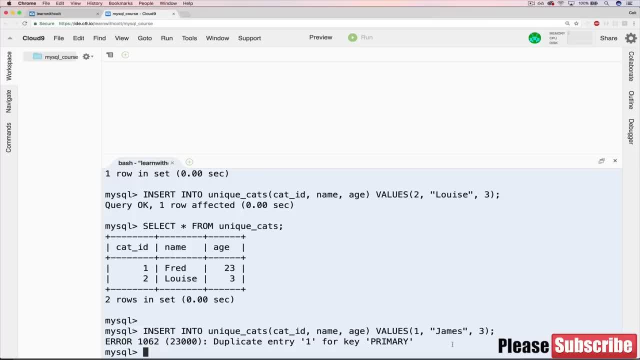 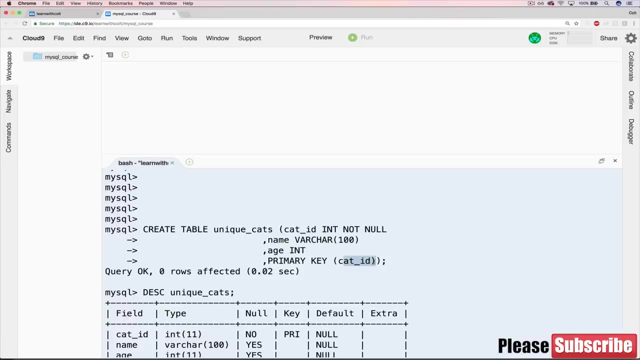 You often want to make a username a primary key, so that you can't have more than one account with the same username in your database, And so all that you would do is, instead of saying primary key- where's that cat ID, you would say primary key, username, or whatever the name of the field is. 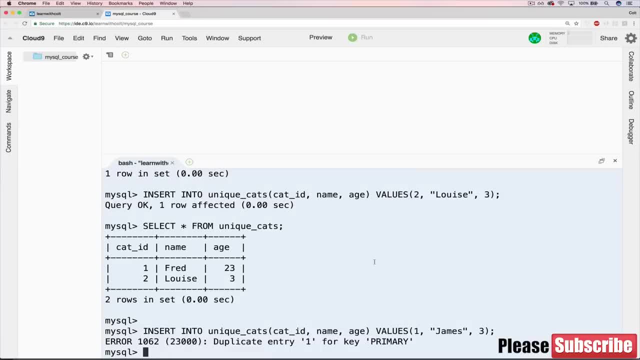 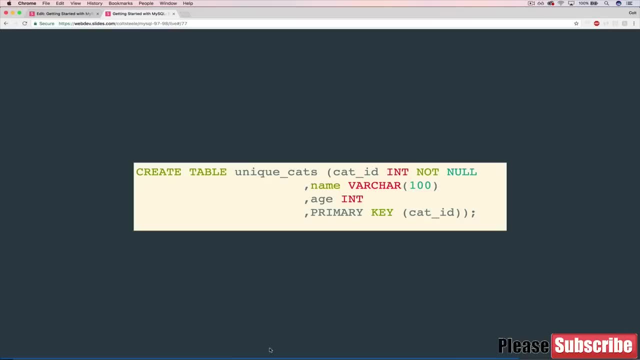 And then if I tried to insert something with an already existing username, I would get the same error here. Okay, One more thing to talk about, which is it's kind of annoying to have to manually specify this ID. It's more than annoying. 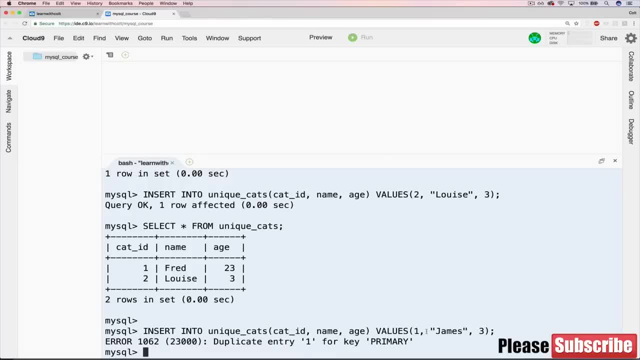 It's impractical. I mean, are you just supposed to know where you left off? One, two, three, And every time you insert a cat you just have to know what the last one was. It just doesn't really work. 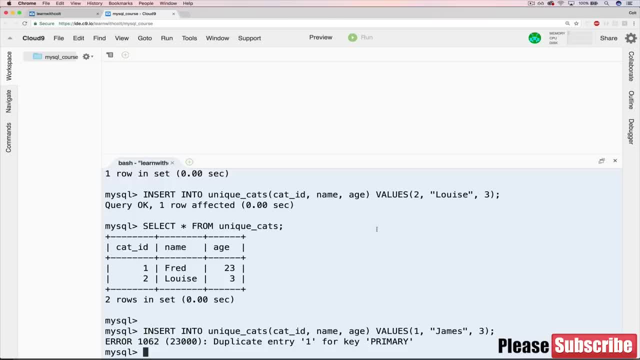 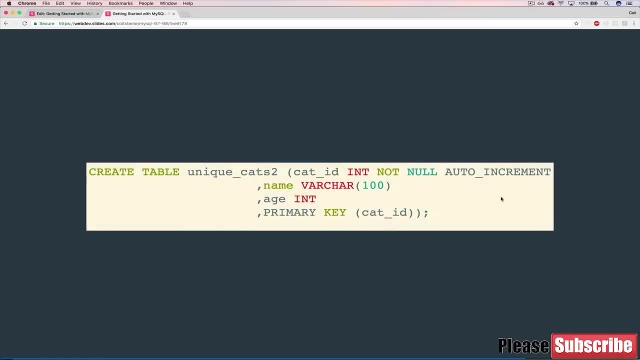 It's not even in this shell context, but especially not in a real application. You can't, and it's just a pain. So there's a way around it. Our code gets longer, I know, but all that's added here is this: auto increment. 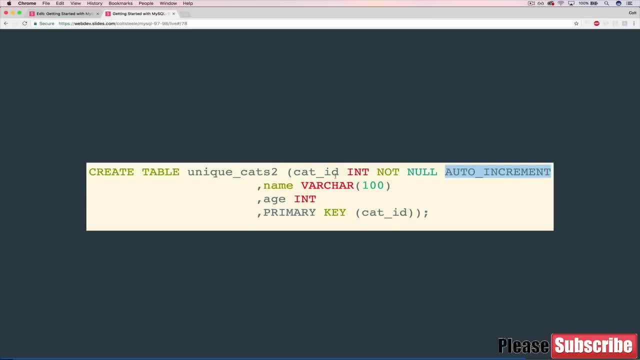 So it does what it sounds like. It will take cat ID and it will automatically add one to it Every time a new cat is created, So we no longer have to specify: cat ID is one, cat ID is two. It will just do it. 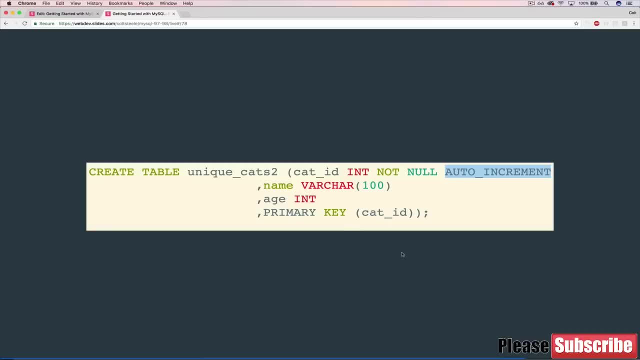 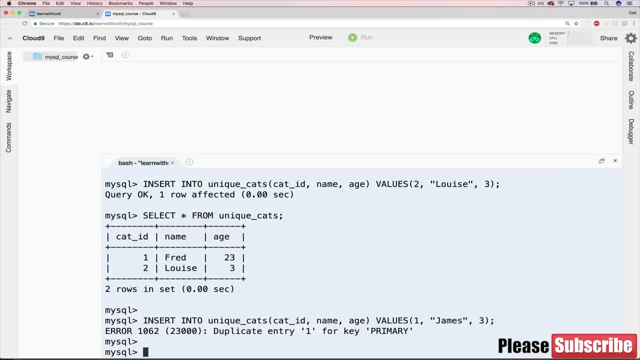 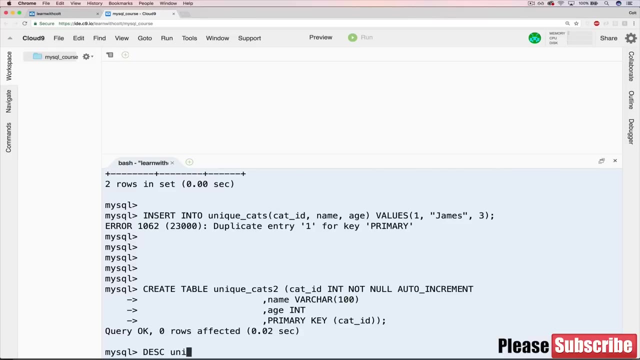 We just leave off cat ID entirely and everything else here is the same. So cat, unique cats too. I'm just going to copy this over, make some space, hit, enter And before I show you that it works, if we do describe unique cats too. 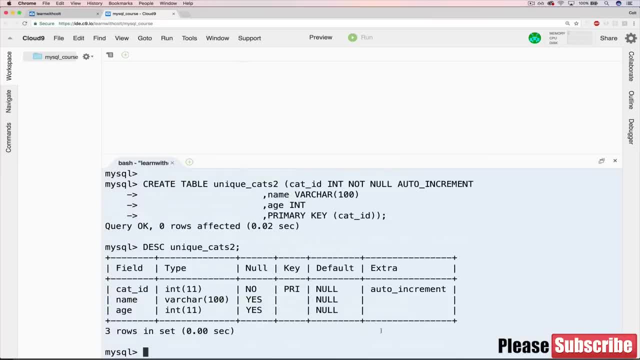 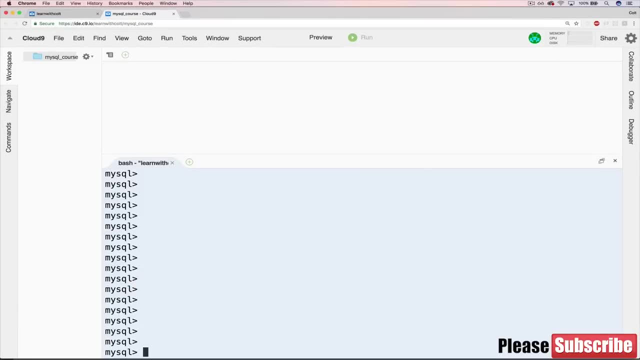 you'll notice that we also have auto Whoops. We have auto increment here under extra, So it doesn't get its own field, but it's considered extra. So now let's try and insert something into that, Insert into into unique cats too. 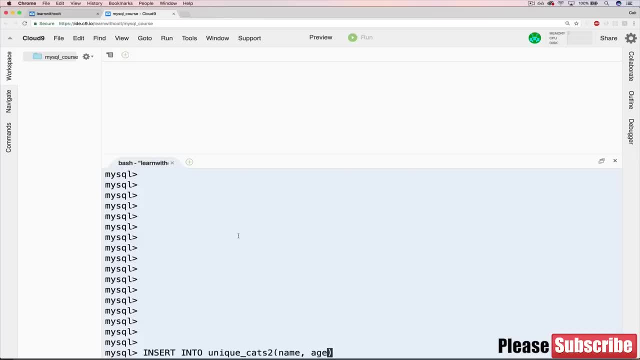 And we'll do name and age. We don't specify cat ID anymore, Values, And let's see Seriously the hardest part of all of this. Let's go with Skippy Once again. I see some peanut butter in my kitchen- and age will be four. 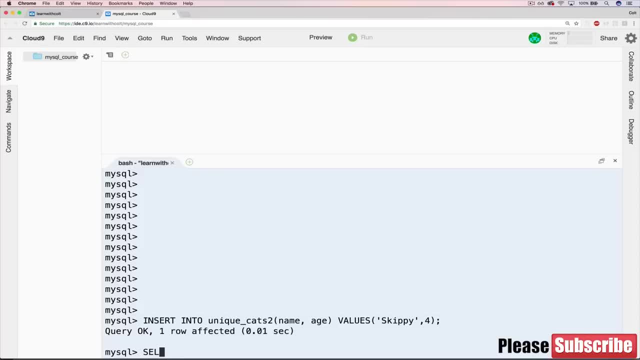 Just like that. Now, if I do select star from unique cats too, cat ID is automatically one, And to prove to you that it's auto incrementing, let's change this name to Jif And we select star again, And now we have two. 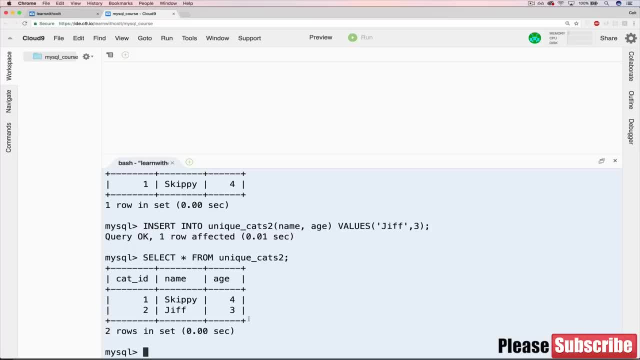 So this solves two problems. One is that it's annoying to have to manually type those IDs and keep track of what number we're on next. But also I can now have duplicate cats as far as name and age, which is our whole goal from the get go. 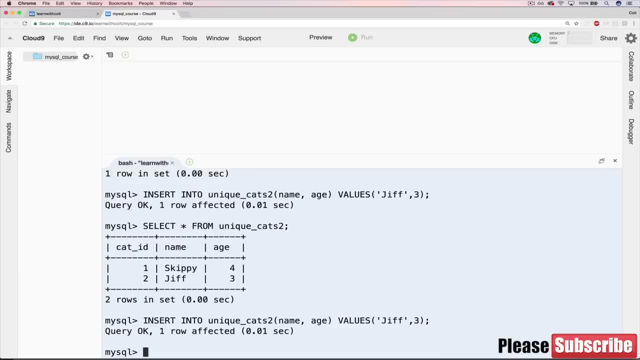 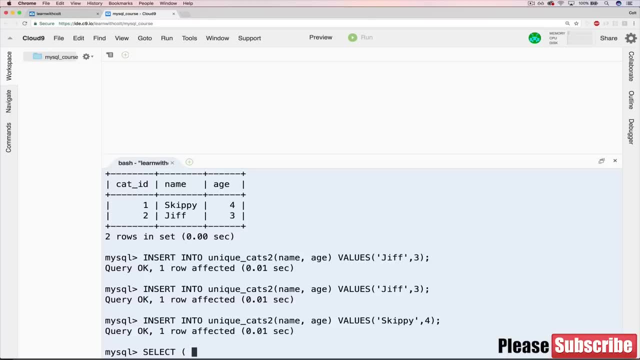 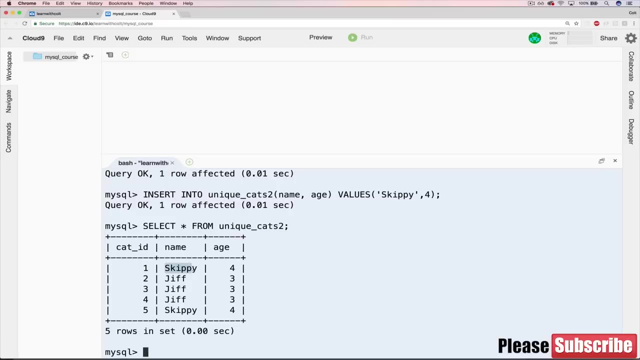 So I can now do another Jif And another Jif again, And this time let's do a Skippy as well. Now select star from unique cats too, And you can see we have Skippy here, who's four and Skippy here, who's four. 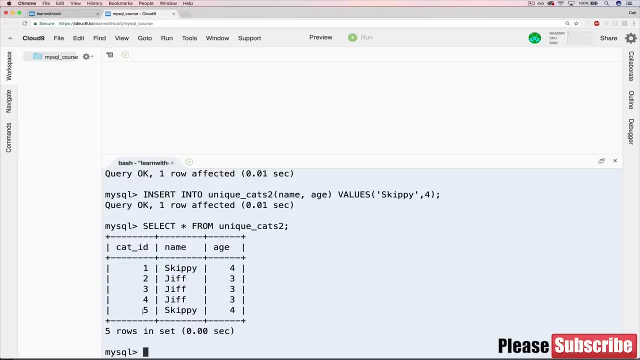 but they have different IDs. Therefore they are unique. Same thing with three Jifs, Perfect Alrighty. So that concludes all the new stuff in this section. Now you're going to get a chance to put in action, to actually practice it and to write your own bit of code. 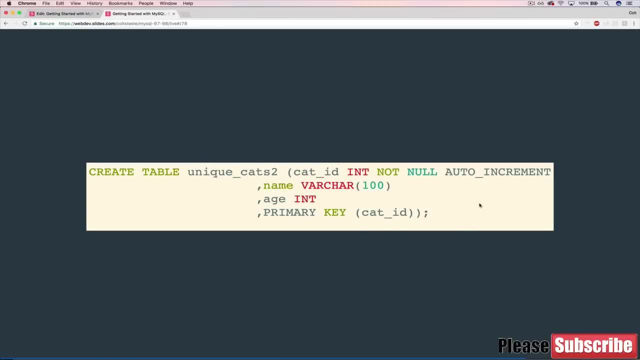 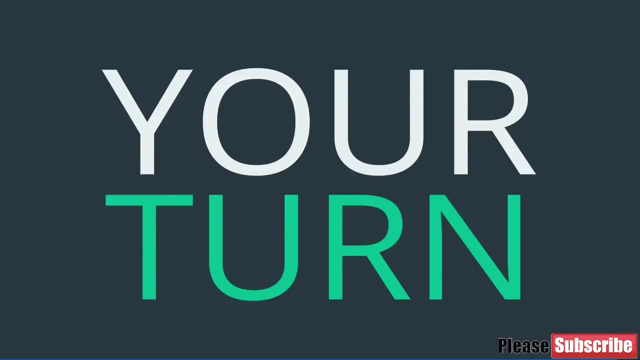 create your own table that looks a little bit something like this: Okay, All right, So it's your turn to put some of this into practice with a single exercise. It should be pretty quick. All you need to do is define a single table. 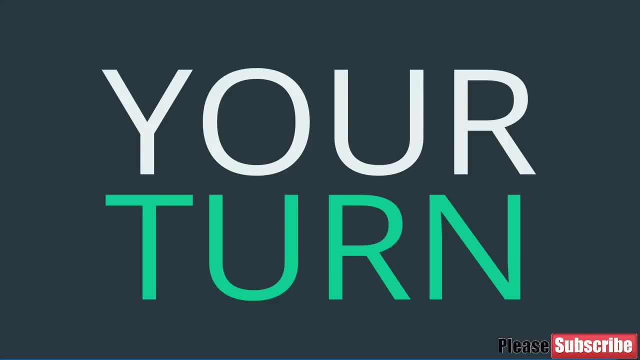 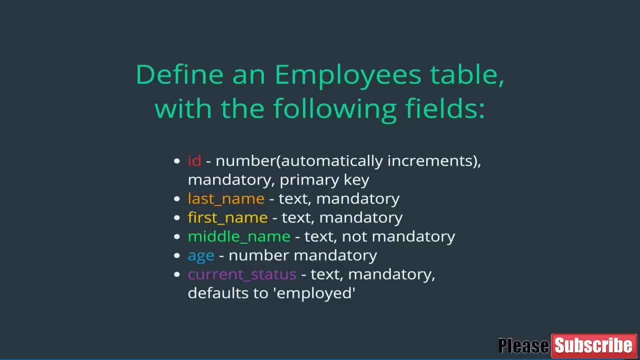 So here are the demands. Well, demand sounds a little strong. Here are the requirements. Define an employee's table. So let's say we're a company trying to manage some employees. We'll definitely need more data than this to actually make it operational. 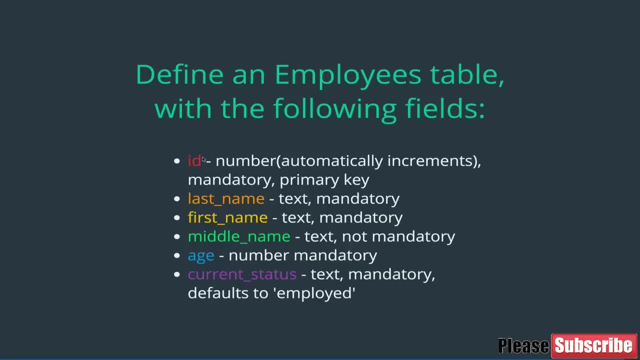 but for now this is all. we need. Seven different fields, seven columns: ID, last name, first name and middle name, And then age and current status, And actually I can't count. This is six, So ID is relatively self-explanatory. 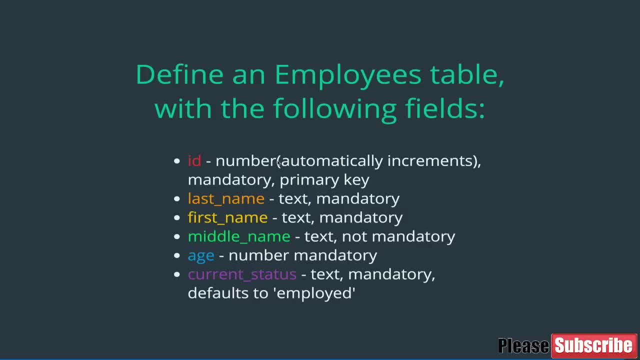 It should be a number. I'm not telling you the data types, but you should know at this point what they are. So a number that automatically increments. It's mandatory, so it can't be left off And it's a primary key. 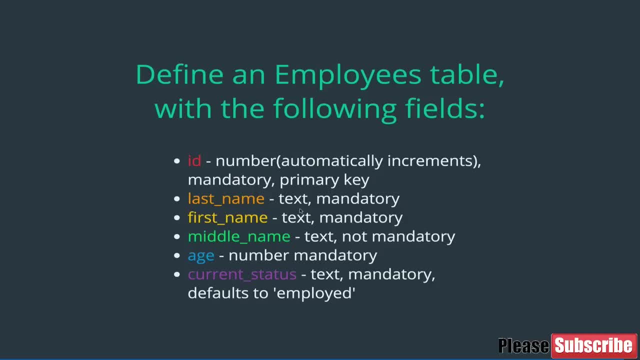 Last name and first name are both text, which isn't a data type. Again, you need to use the actual term, And then neither of them can be left blank either. They're mandatory, But middle name while it's also text. 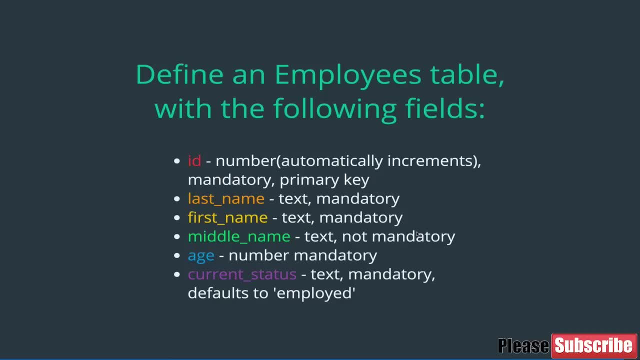 it isn't mandatory because not everyone has a middle name, So we can leave that blank. Then we've got age, which is numeric and it is mandatory, It can't be blank. And finally current status, which is essentially like their employment status. 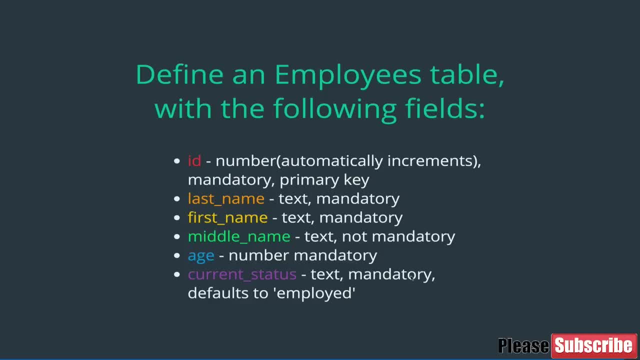 if they're employed or if they're fired, And it should be mandatory, so it can't be null. But if no status is provided when something is inserted, it should default to employed. So we'll have two statuses: employed and terminated, or fired or something. 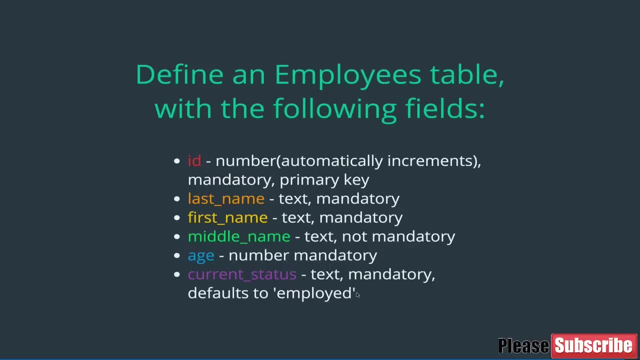 I guess terminated is more professional And so it should just default to current status: is employed, If nothing is provided when it's inserted. Okay, so go ahead and define this table, type it out, try running it to make sure it works. 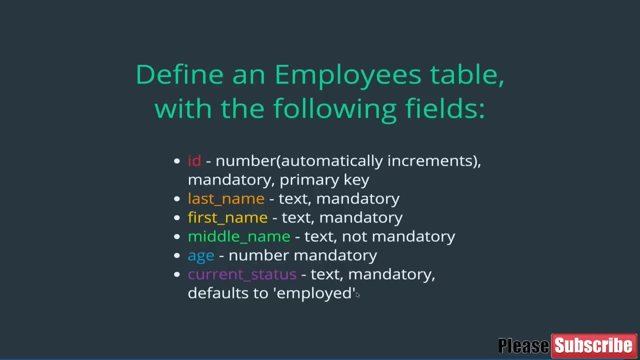 and then try inserting some data as well to make sure that it works. Okay, If you want a solution, have it in the next video, All right. So if all you care about is the solution, just check out the code following this lecture. 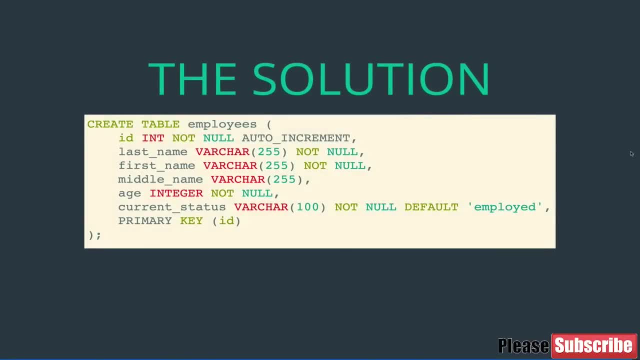 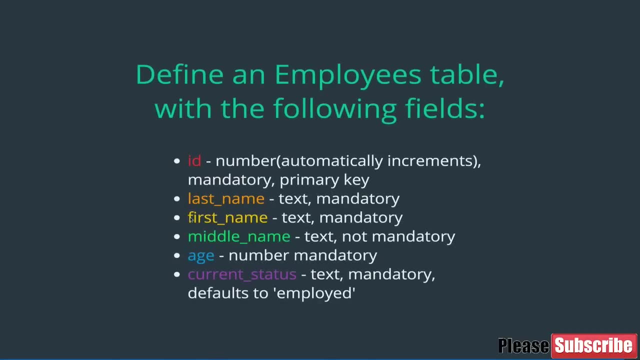 or pause the video. You can see the solution here. But I'll go ahead and go through the process of typing this out very quickly. I'll kind of speed it up. So what I like to do is start by defining the rough skeleton of what we need in a SQL file. 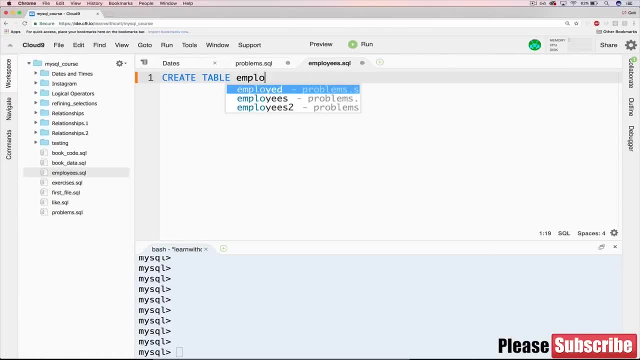 So we need a create table employees And then within that we'll have ID, We'll have first name, We'll have last name, We'll have middle name And then we have age and current status, just like that, And then we can fill in the data types. 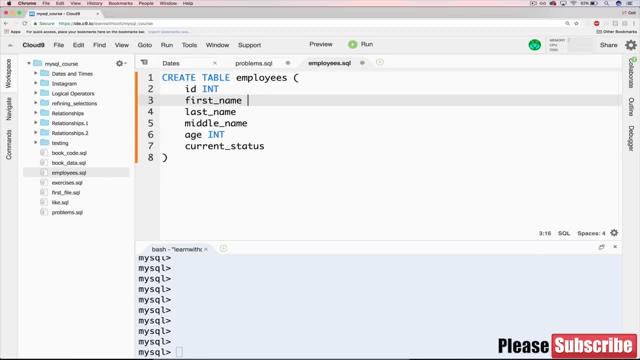 So we know ID is an integer and age is an integer, And then these are VAR chars for our cars, Let's say 255.. Somebody may have a giant name, And same for current status. So then, the next thing that we could do, 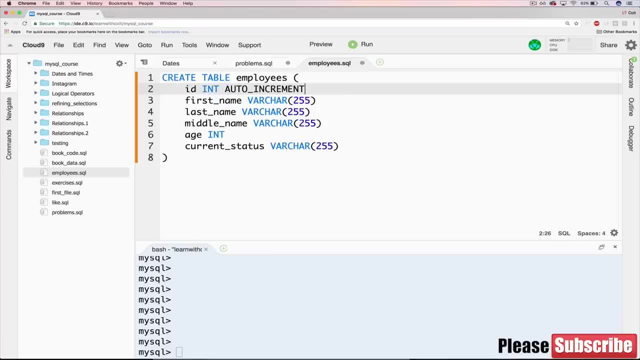 is focus on ID, which we know needs to auto increment, And we also want it to be mandatory and a primary key. So mandatory means not null, And a primary key. there's actually two options. The first one is to do this. 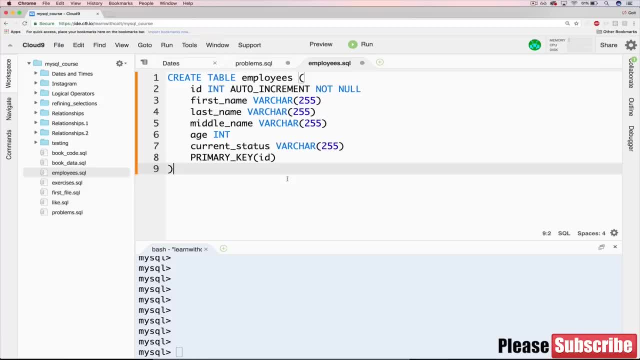 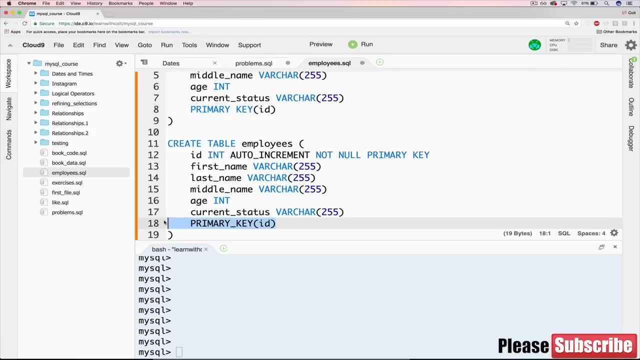 And the second one just duplicate. this- it's also in the slides- is to add it on the end here. We don't want that underscore there. There we go, So these will do the same thing, But of course we're not done. 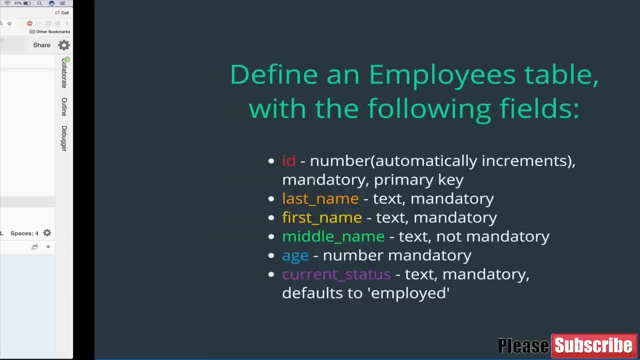 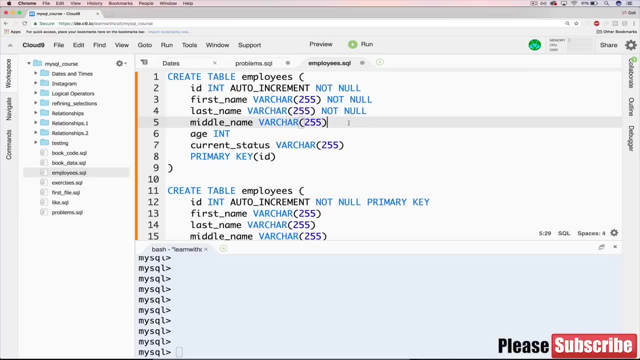 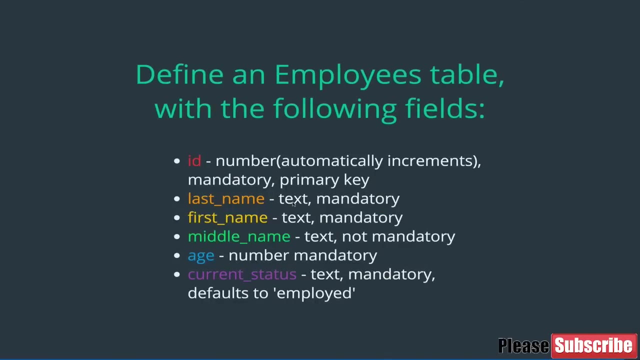 So the next thing would be first name, And first name is just mandatory, as is last name. So we'll just add not null and not null Middle name. we can leave alone. Then we've got age, which is also mandatory, And then finally, current status. 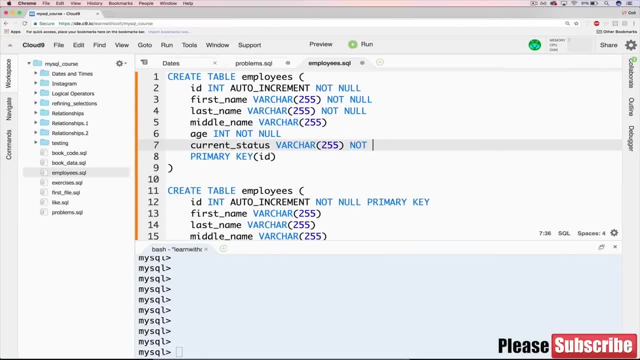 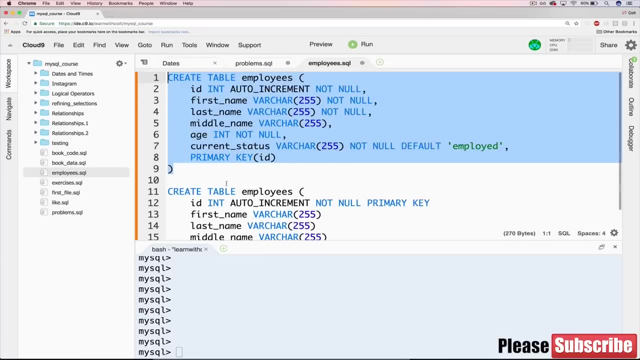 which is mandatory, but there's also a default value, So we want not null default employed. And then we need to make sure we have all of the correct commas here, Just like that. Add our semicolon as well. Copy it. 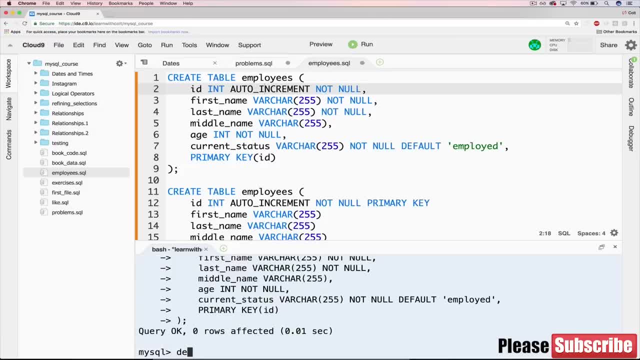 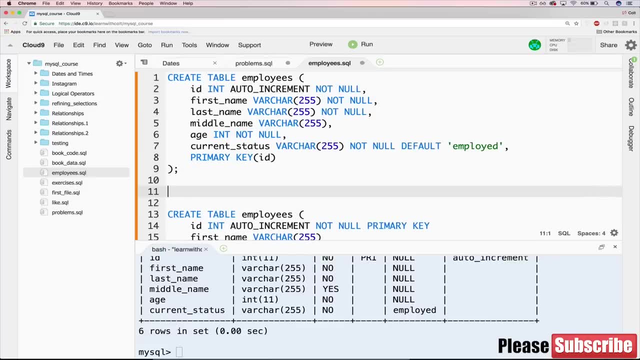 Let's see what happens. All right, so it looks good, We can describe employees And then, if we wanted to, let's just do a single test insert to make sure our default value works and our auto increment works. So we'll do insert into employees. 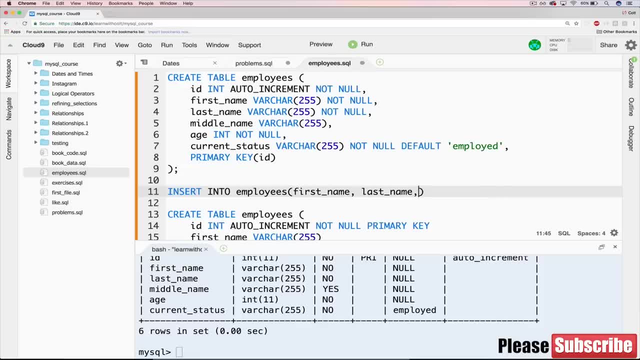 And we'll do first name comma, last name comma, age, And that's it, because everything else either is allowed to be null or has a default value, And we'll insert someone with the name of Dora Smith, I guess. 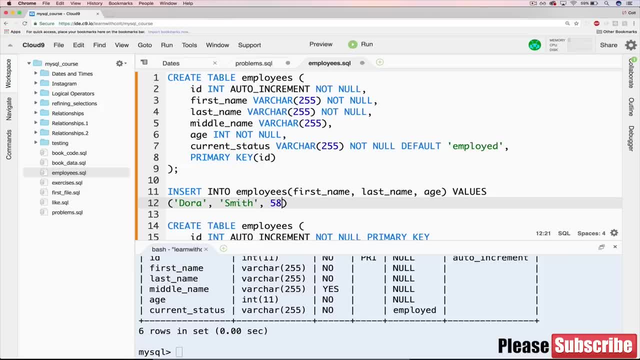 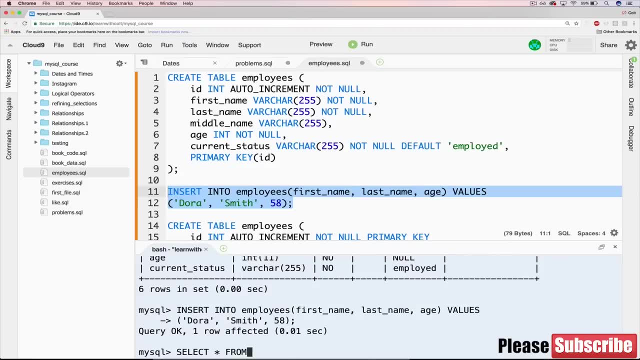 And let's say she is 58.. Okay, Copy that, paste that in. Let's do a select star from employees, Just like that, And it looks good. We've got an ID auto incrementing at one first name, last name. 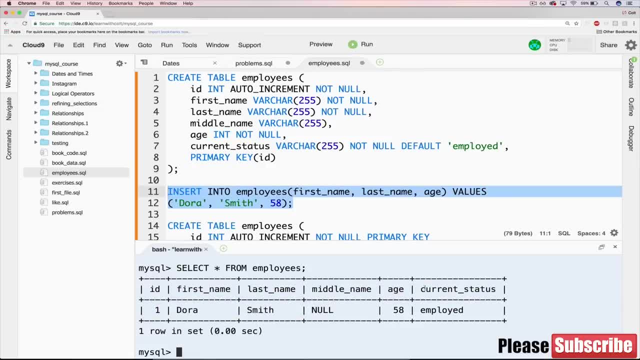 middle name is null because it's allowed to be. Age is 58. And current status is employee because we didn't specify one and we have a default value. All right. So again, the other solution here is just to put primary key on the same line. 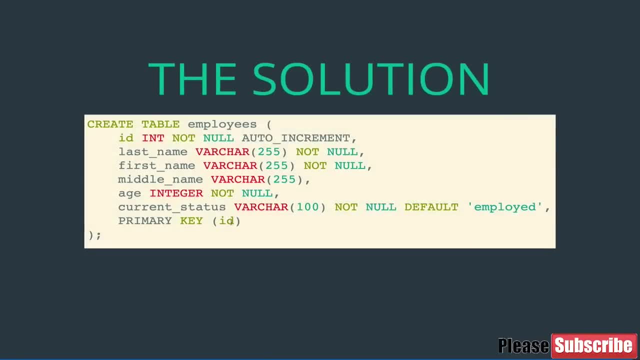 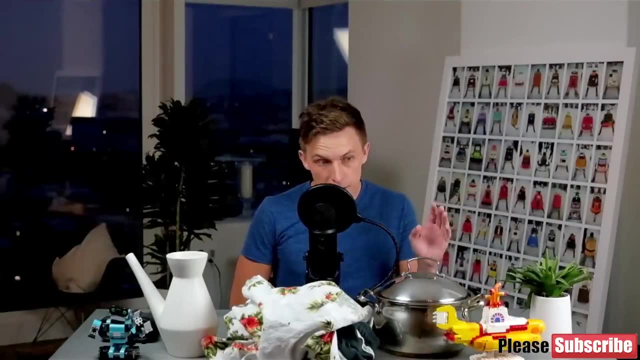 when you're defining the column. I prefer to do it that way, but you'll also see it done this way. Both work All right. That's it. Hey, welcome back. If you're looking at my desk right now and you're asking: 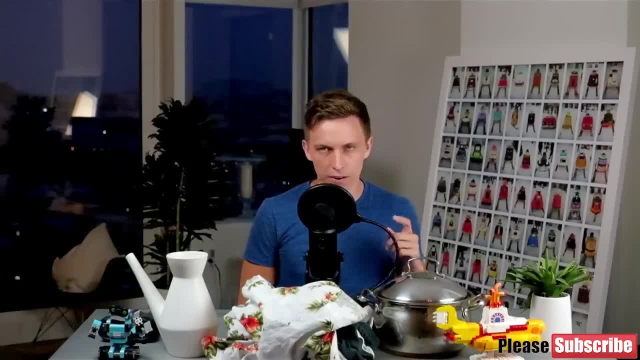 wow, why is there so much crud on it? Well, you're onto something. This section is all about crud, Yeah, So crud is an acronym. It stands for four things: C, R, U and D, Create, read, update and delete. 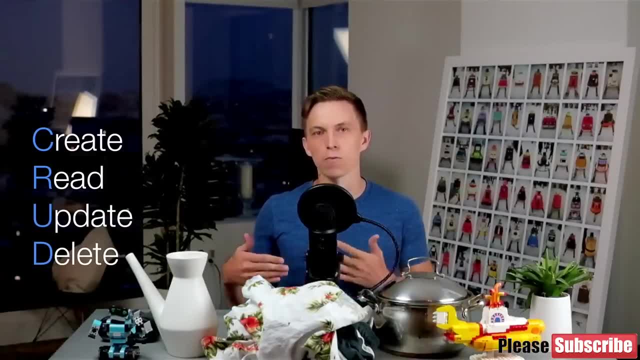 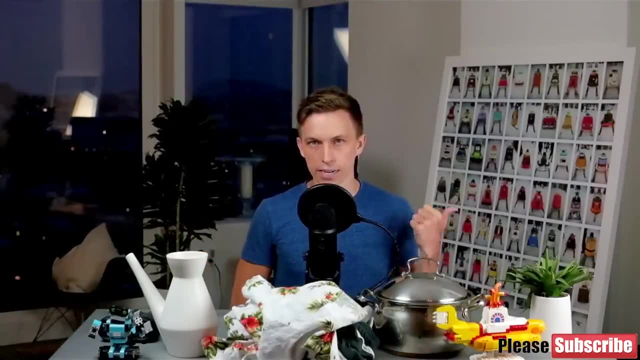 And they are the four basic actions that we want to be able to do to our data. So we've actually seen two components already. We've seen how, let's say, we're working with users. We've seen how to create users with the insert command. 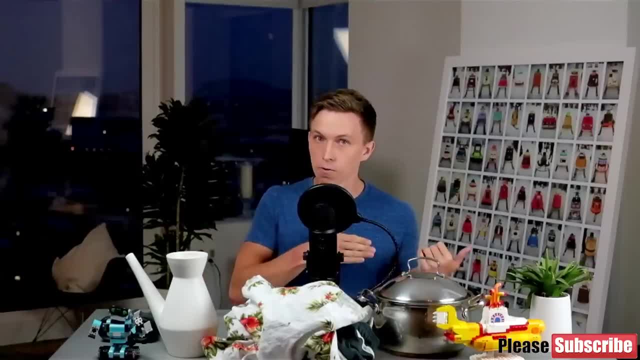 We've seen how to read users, take them back out. you know, spill the milk out of the database. That is the read section, which we did with select. Now we also are going to review more about select and insert, but primarily we're going to see: 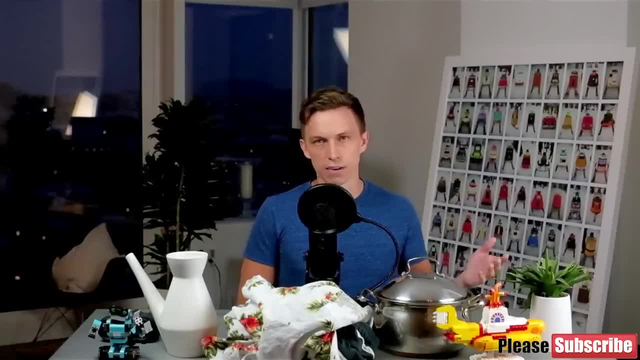 how to update and delete information. So how do we change something in our database? if we made a mistake, or let's say a user changed their password, They clicked a forgot my password link and they want to reset it, We need to change it in the database. 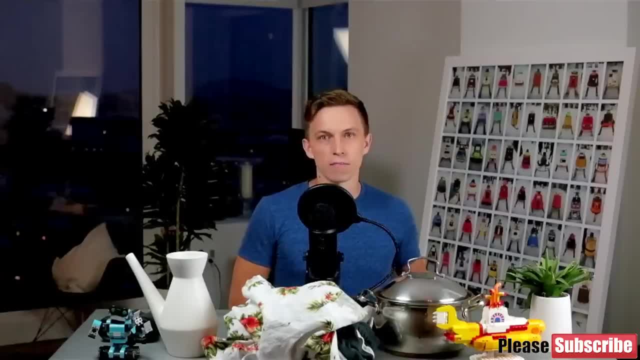 and then delete. Let's say, our user decides to leave our site for some really bad reason, We can delete him or her. So that's the focus of this section. We're going to have a ton of exercises because we're seeing a lot of commands. 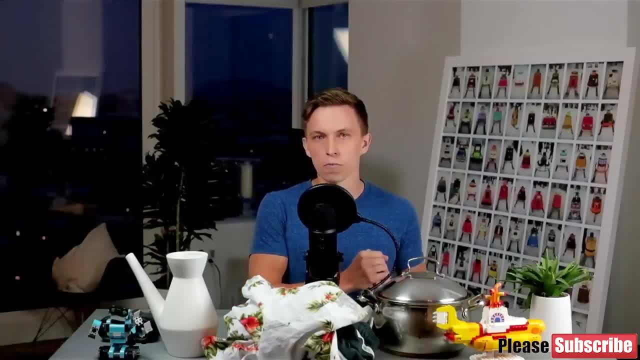 and now that we have those four commands in place we'll be able to go do a lot of stuff. They're kind of the fundamental four things of any database or any data. So tons of challenges coming up. Look forward to that and I'll see you basically in the next section. 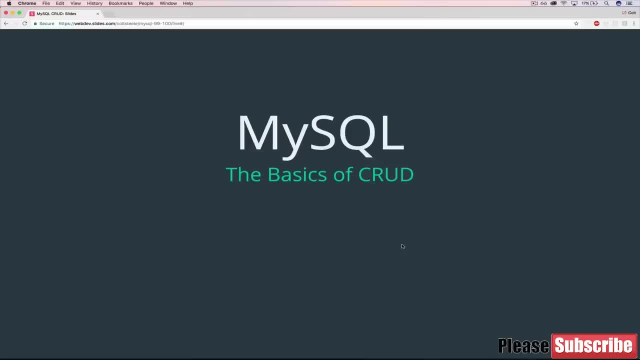 when I have to do another one of these videos. See you in a bit, Alrighty. So in this section we're going to focus on the basics of something called CRUD. So it's an acronym: C-R-U-D, and it stands for create, read, update and delete. 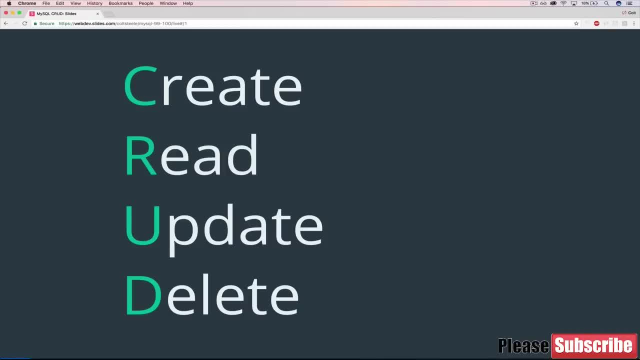 or destroy some variation of that. The idea is that these are the four main operations that we perform on our data. We've already seen how to create data. When we have a database, we want to be able to add data in. We want to be able to search back. 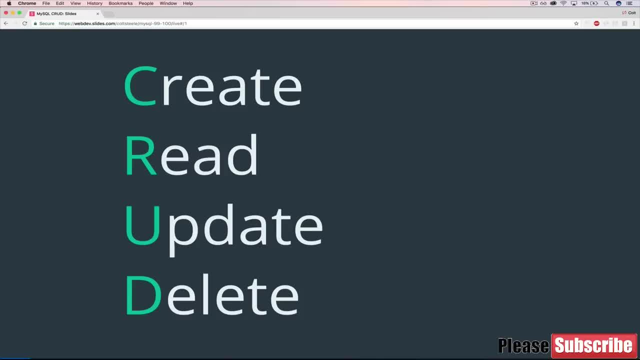 or read it back out. We want to be able to update it and then also to delete it. Those are the four most important and most common operations that we'll do In CRUD itself. the acronym is not particular to databases. It's common in other facets of programming. 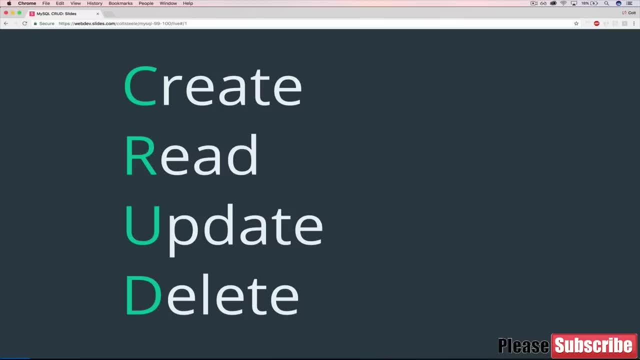 and web development, but it's a nice acronym that fits what we are trying to do here. So what we're going to do is step through all four different operations, And we've already seen create. It should be review, hopefully, which we do using, insert into. 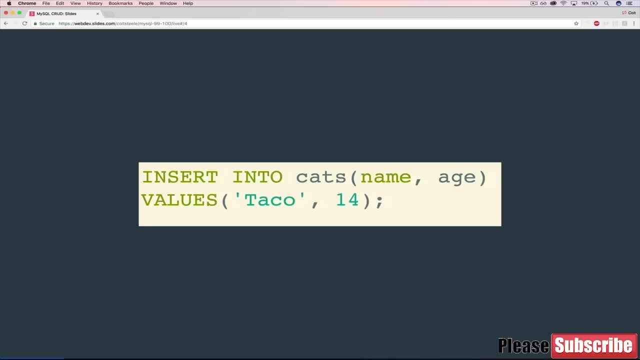 So, going back to our cats, we have things like insert into cats name and age and then the values taco and 14.. So we won't spend any more time talking about create in this section, but we'll be using insert into 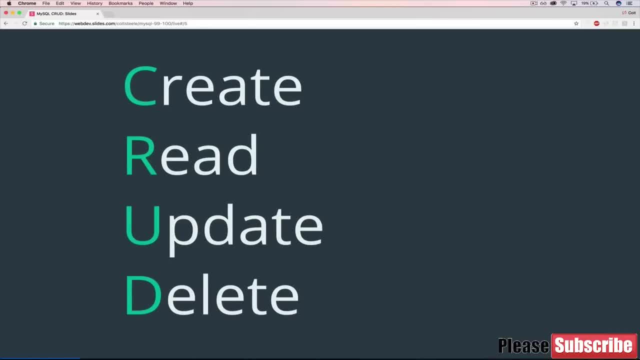 throughout the rest of the course, But really, what we're going to focus on here are the other three operations. So how do we read data out? How do we search? How do we find things? How do we update data If we made a mistake? 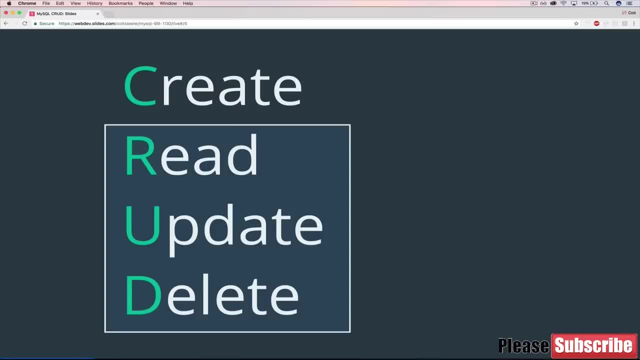 or something changes, and then how do we delete data, How do we delete everything from a table And how do we delete one or two things at a time? So that's really what this section will focus on And we'll kick it off. 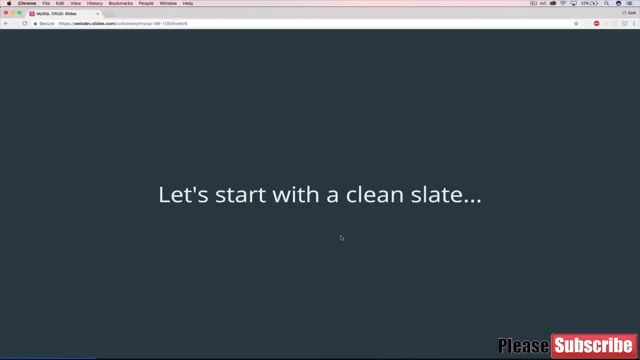 by talking about reading data out. Okay, so before we see any new code or new commands, I want to clean up the data that we currently have. If you remember, we kind of added a bunch of different cats databases. We have cats and cats one. 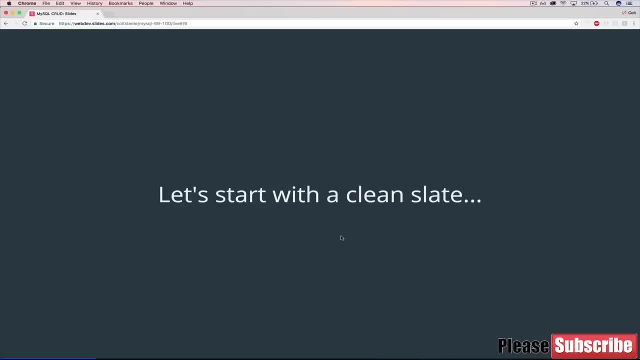 and cats two and cats three and so on. What I want to do is delete the original cats table and then we're going to remake it, but with a few additions, because our original cats table was the most basic. It only had name and age. 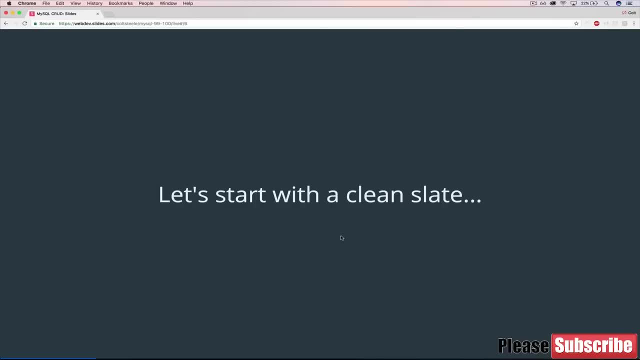 but I want to add some other data in, like an ID that auto increments and so on. So basically, we're just going to remake the cats table and add new data in. So if you want to make a bit of an exercise out of this, 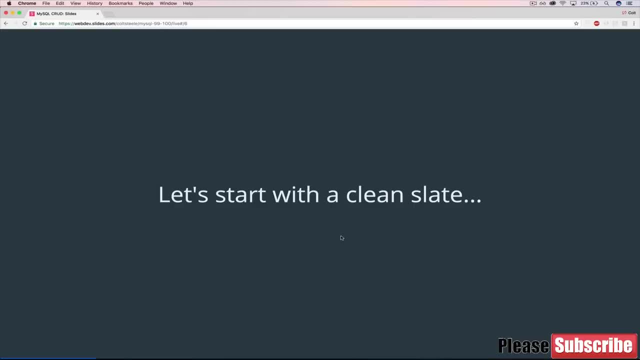 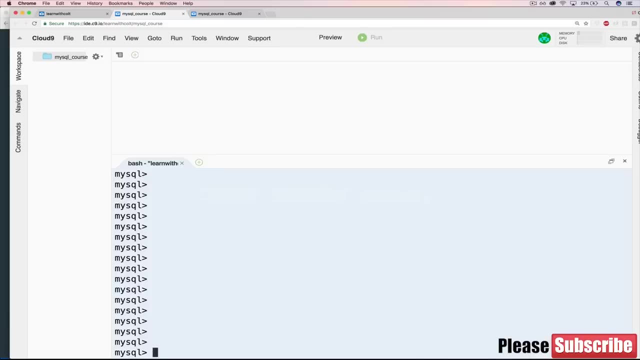 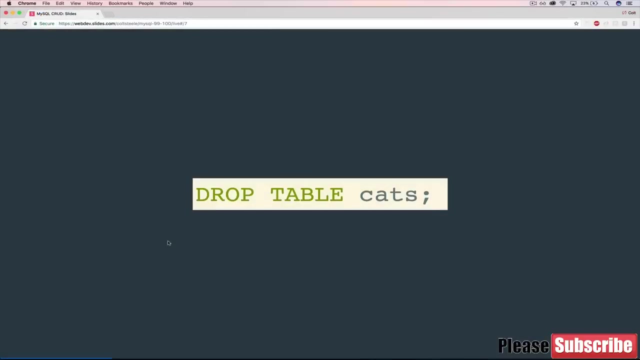 the first step would be to delete the cats table. So do that now. And the command, if you want to see it, is: drop table cats. So let's do it. Drop table cats. Oops, There we go. And now that we've dropped the table, 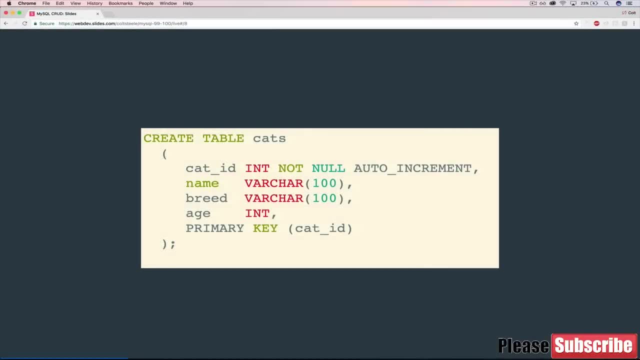 we want to recreate the table, So this is what we want here: We're going to have a cat ID integer, not null auto increments. We're going to have a name that's a varchar, a breed that's varchar as well. 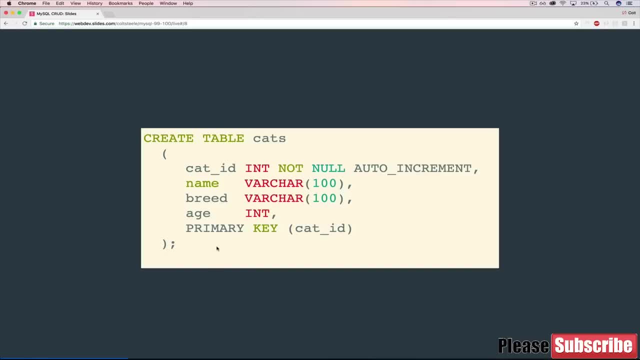 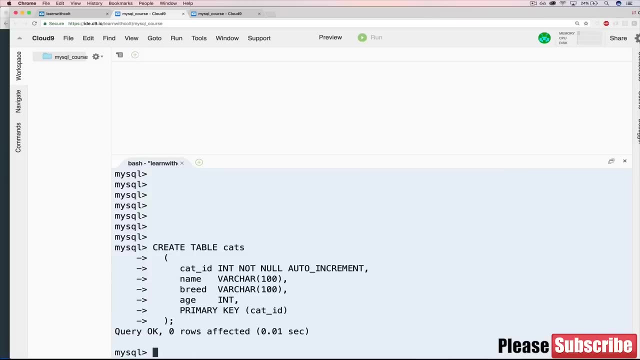 an age. that is an integer and cat ID is our primary key. So if you'd like go ahead and type that out or just copy it, paste it in Perfect, Of course we could make sure it worked. Describe cats. 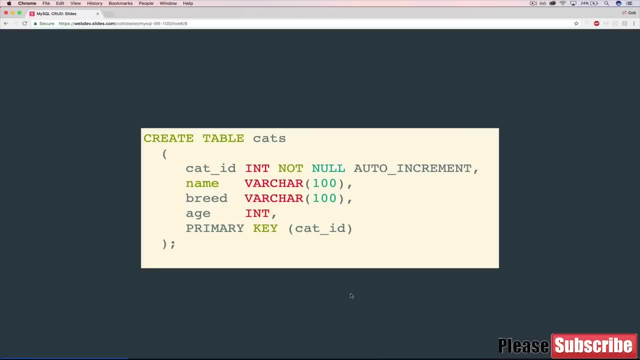 There we go, All right. So the last step here is to add new data in, And I would like for you to have this same data, because we're going to use it throughout this section. There will be a couple of activities and questions, and it will be much easier. 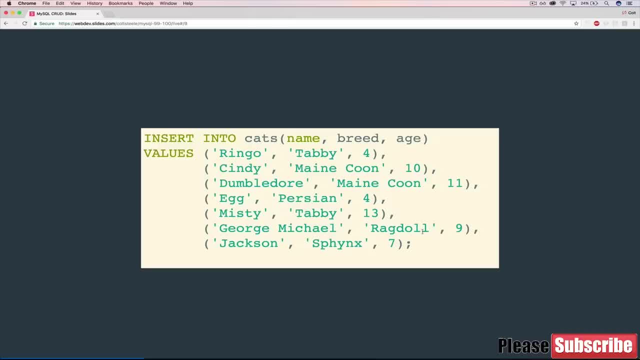 if you have the same data as me. So we've got one, two, three, four, five, six, seven, eight, nine, 10,, 20,, 21,, 22,, 23,, 24,, 25,. 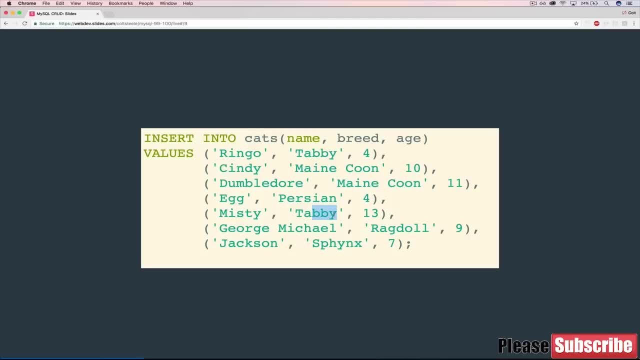 26,, 27 cats. Each one has a name, a breed and an age. Some of them. there's a couple of Maine Coons, a couple of Tabbies and a couple that have the same age, which we will use. 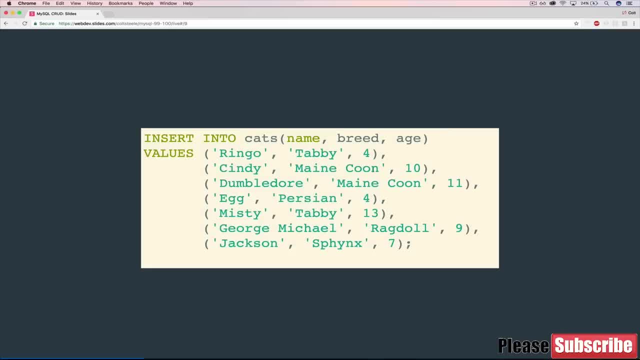 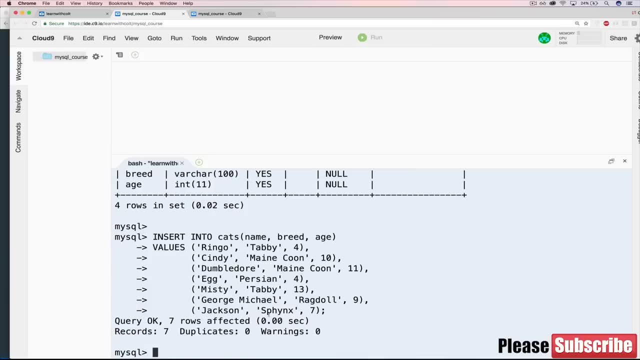 in just a little bit. So copy this, or, if you're a masochist, you can type it out, Paste it in Perfect. And now we have seven cats in our database, Seven rows, Okay. So now we've prepped our data. 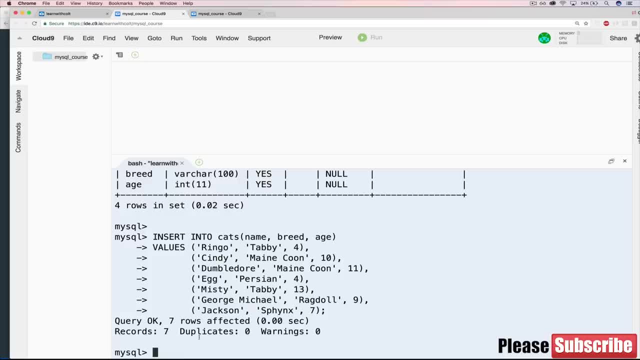 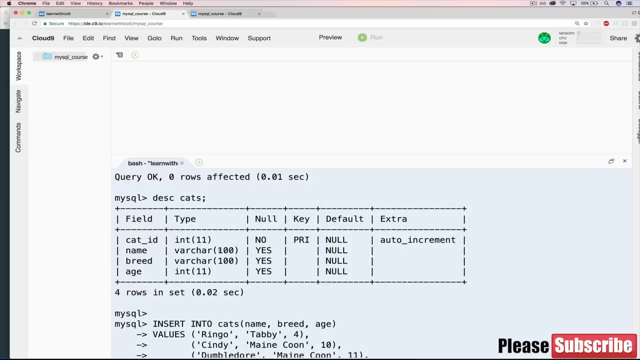 and we're ready to go. So we're going to go to our database and we're going to go and we've deleted the original cats table, remade a new special cats table with some more interesting pieces of data and then we've inserted data. 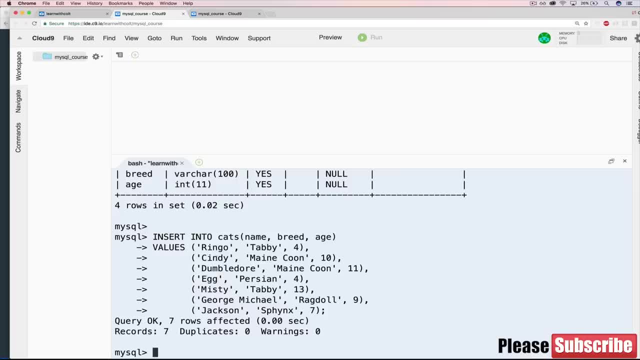 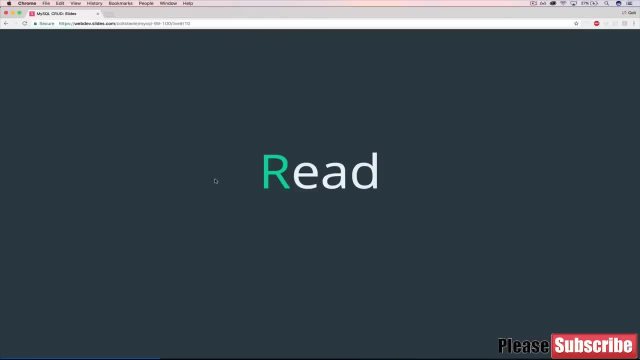 in there as well, Awesome. Next, we're going to move on to talking about searching or reading data out. So we're moving on to the R of CRUD, which is read: How do we retrieve and search data from a database? And we've actually already seen this. 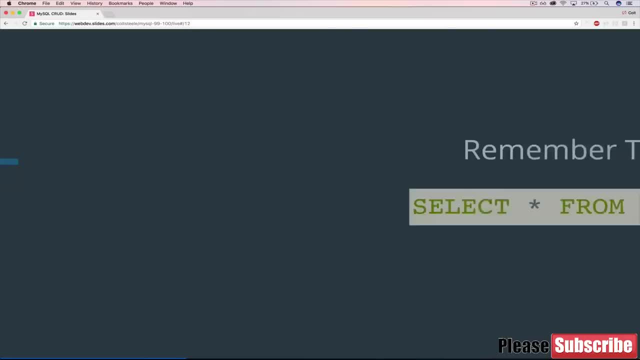 The magic command is select. So remember when we were doing this earlier- select star from cats- I told you not to worry about it too much because we'd spend more time on it And it was really just something that we needed to have to check our work. 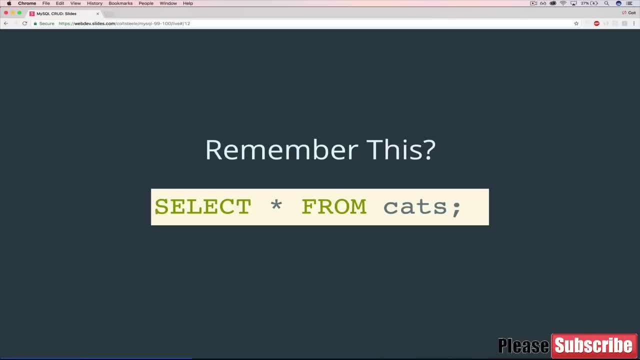 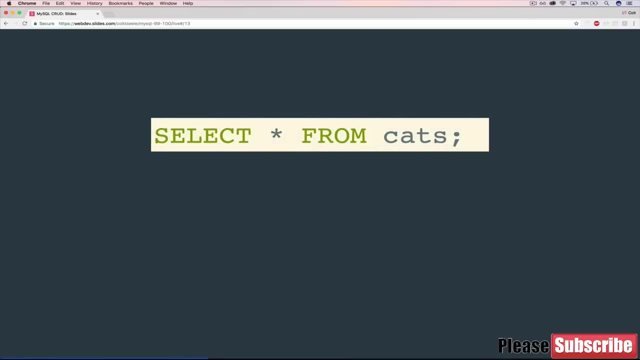 at that time when we were inserting data, But we didn't actually talk about how it works, what the star means. That's what we're going to do now. So the star in select star from cats means: give me all the columns in the cats table. 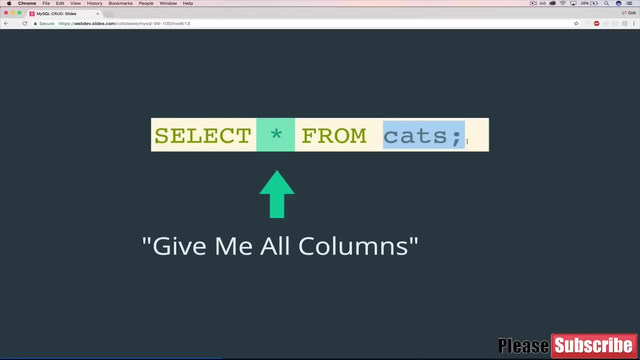 So we're asking for the cats table. That's the from cats, And in that table we just want everything that we have. So in our case that means cat ID, name, age and breed. We want all of them coming back to us. 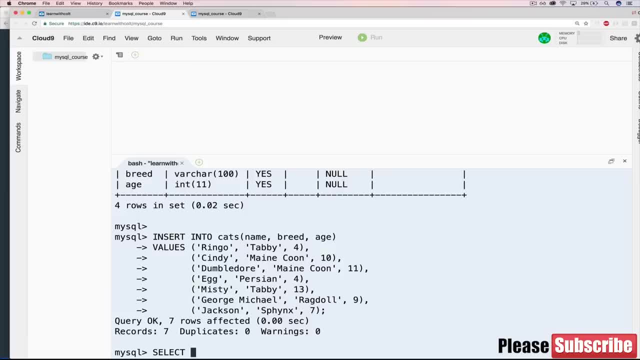 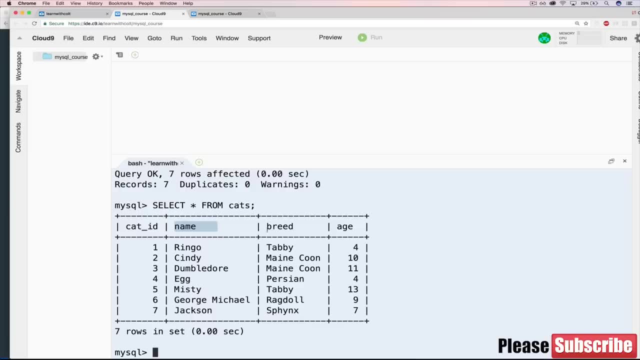 So let's do that now. Select star from cats. You can see we get cat ID name, breed and age And we also get every single cat. No one is missing. These are the seven that we inserted, So that's the basics. 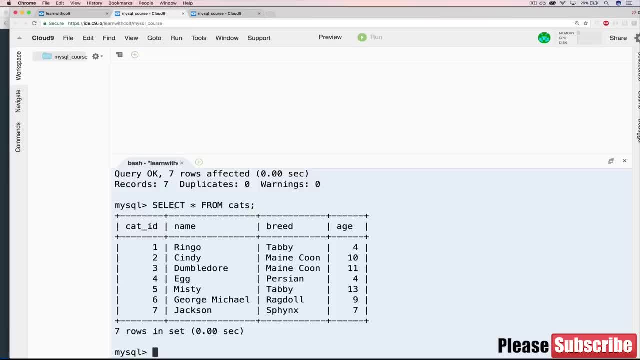 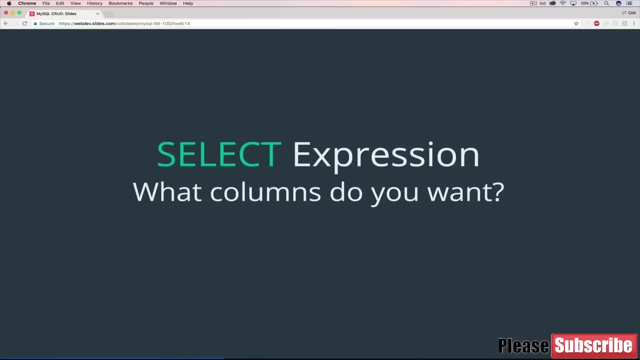 of select star, which you'll use often just to check things out, But we can also get more specific about what data we want back, which is where the select expression comes in. Basically, there's a way for us to specify what columns we want. 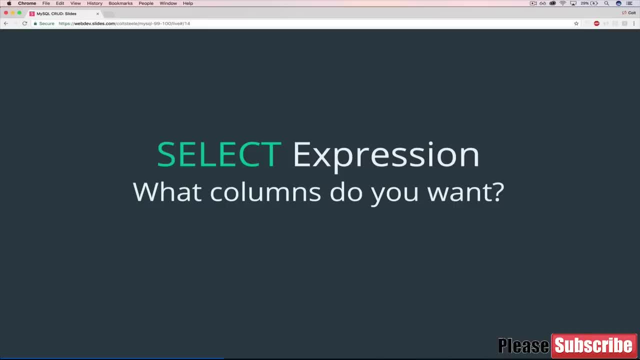 in particular, I only want the ID, or I only want cat's names and age, but not the breed. So to do that, rather than saying select star from cats, we can do things like select name from cats. And if we do that, 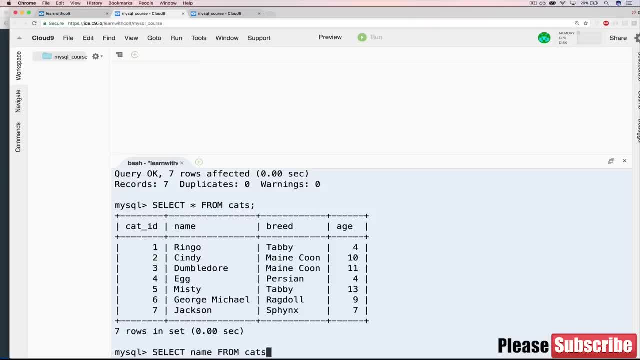 select name from cats. what do you think the table will look like? It looks like this: We only get name, So it gives us all seven names, but nothing else We could also do: select age from cats, And hopefully this is what you expected. 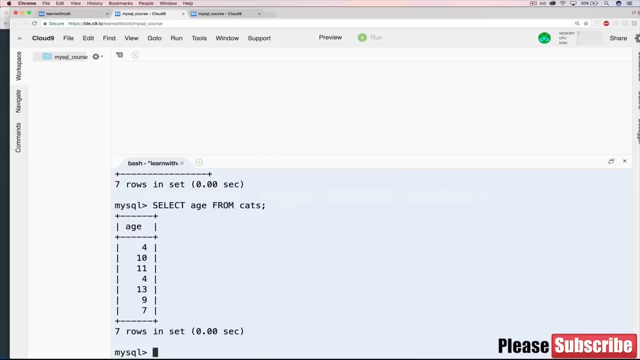 We just get a bunch of ages. And just to hammer it home here, we could also do a select. let's do cat ID from cats, And we get one, two, three, four, five, six, seven. Okay, So that's useful enough. 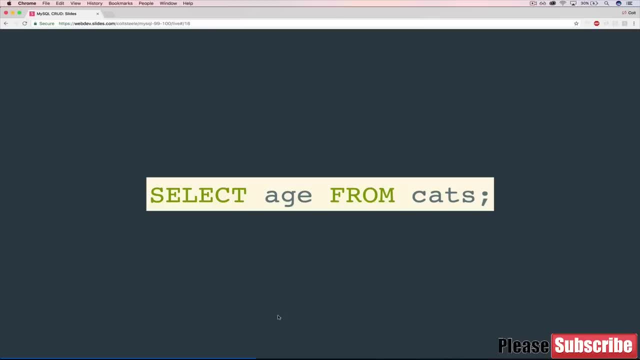 But oftentimes we want more than one piece of data, but we don't want everything, And that's where this comma separated list comes in. So this whole thing is the select expression. We're saying select name and age from cats. So we can try it now. 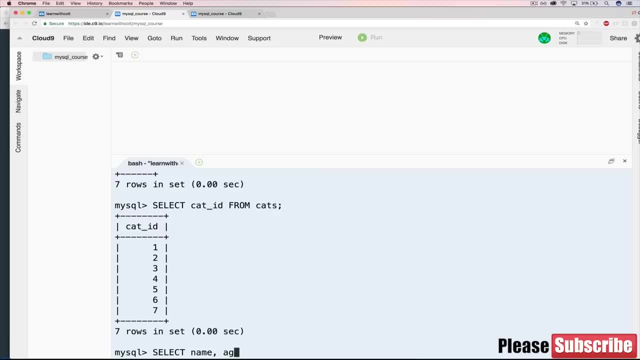 Select name comma, age from cats And what do you think we'll see? So we get a table with name and age returned back, So there's no limit on that. We could do name, age comma, cat ID comma, breed. 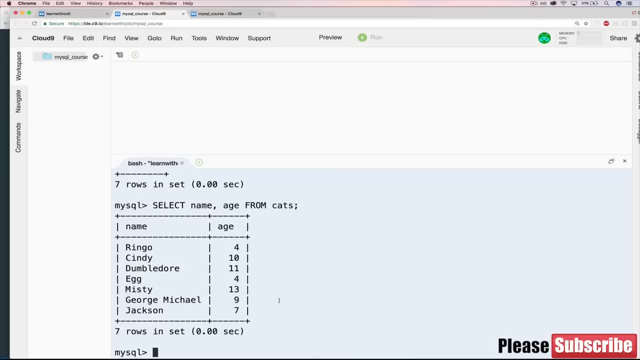 which would be the same thing as select star. We could do name, age and breed or cat ID, comma, breed and name and age, and so on. I think you get it. We can mix and match whatever fields we want back. 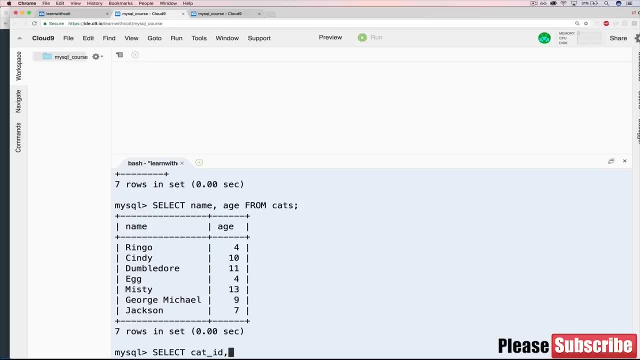 So just to illustrate my point, let's do a select cat ID, comma, name, comma, age from cats And we hit enter And we get those three fields. Notice we're missing breed, But we could just go add that in if we wanted. 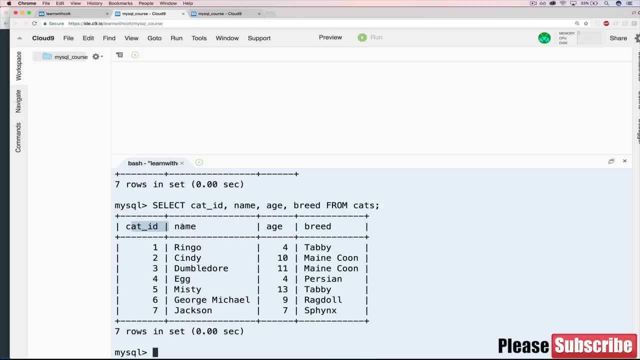 And notice that the order matters. So I said cat ID, then name, then age, then breed, And that's what we get. But if I just did a select star, it uses the default order, which is cat ID, name, breed. 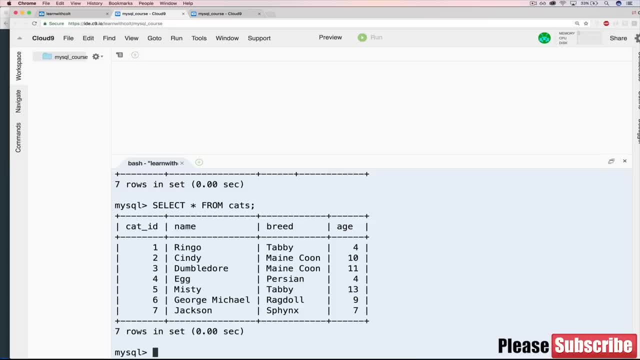 and then age, which is just how we entered it when we created the table. So I could reverse it if I wanted to. I select age, then breed, then name, then cat ID from cats, And there we go. Okay, so that's pretty much. 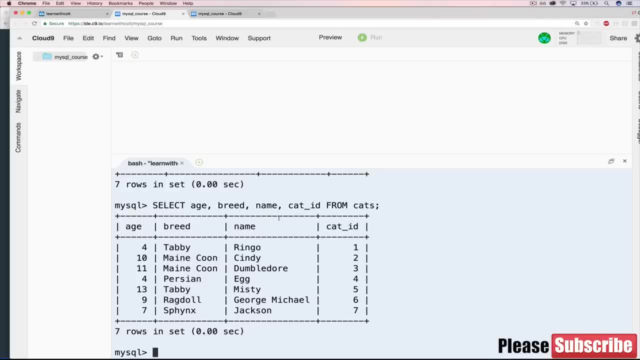 all there is to the select expression, for now at least, where we're just specifying exactly which columns we want, Or we can default and use the star, which will give us all columns. Okay, so what we've seen so far allows us to specify what columns we want. 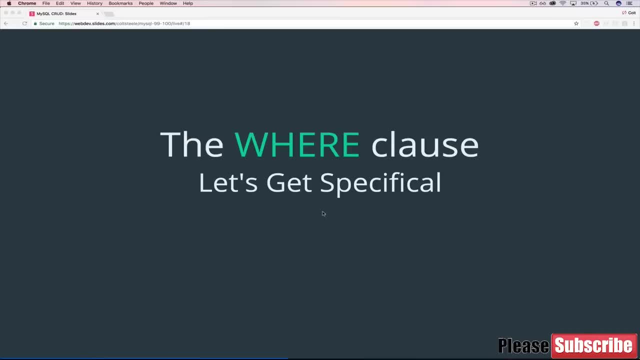 name and age only, or only ID, But it still gives us every single result in the table. So if we have 10,000 users in our database, if we wanted to select one, we don't have a way of doing that right now. 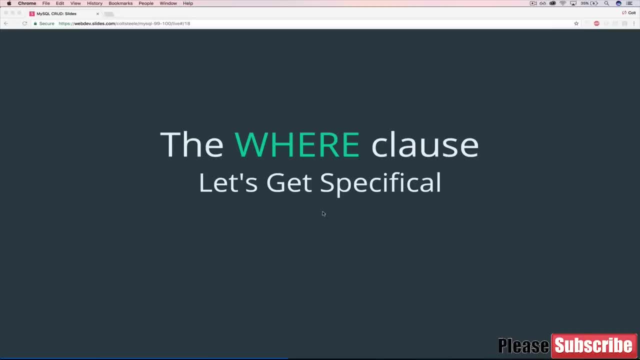 We only can select all of them, which really is not that useful. And in fact, most of the time when you're selecting things, you're doing it deliberately and you're trying to find particular pieces. You're not just trying to check in on your table. 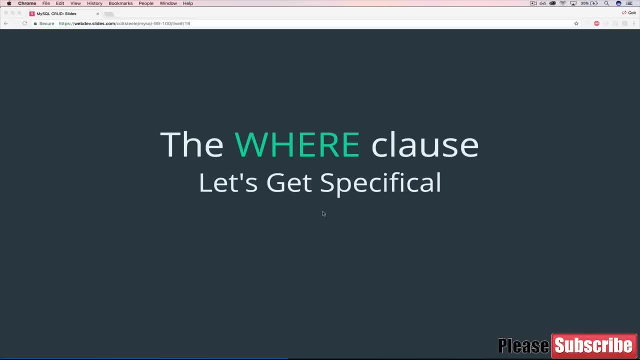 make sure everything's okay. You're usually trying to, let's say, sign someone in. if it's an application, You're trying to verify, find someone by their username and check if their password matches that they entered into your website, or something like that. 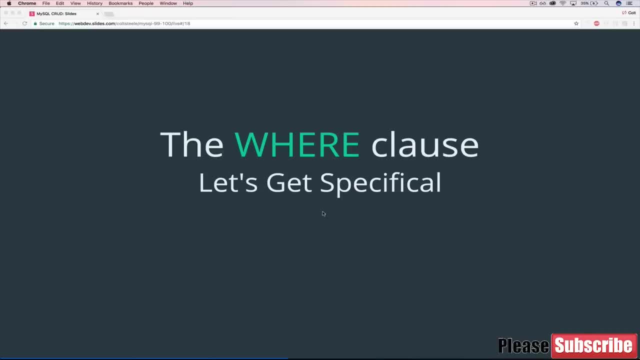 where you're searching for specific data, And to do that, we need to use what's known as the WHERE clause. So it's another magic keyword, WHERE, and it allows us to get specific. It allows us to say: I want all cats who are four years old. 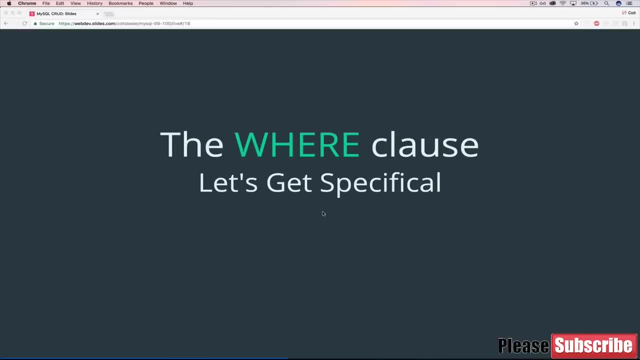 or I want all cats who are tabbies. And those are very simple examples, But later on throughout this course, we'll continue to expand your arsenal for select and for searching. You'll be able to do things like I want all cats that are tabbies. 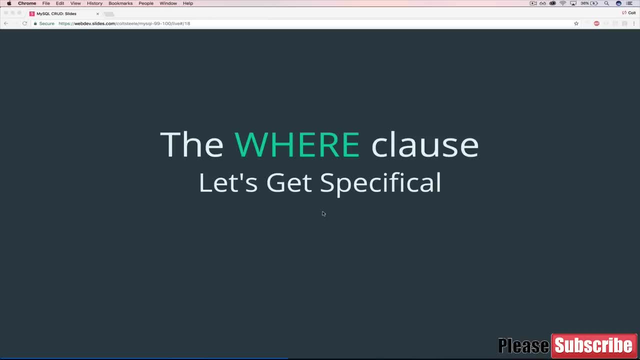 between the age of one and two and whose name starts with the letter B. let's say So. we'll be able to get much more specific, But for now, we're focusing on the basics And, as a side note, I want to show you that 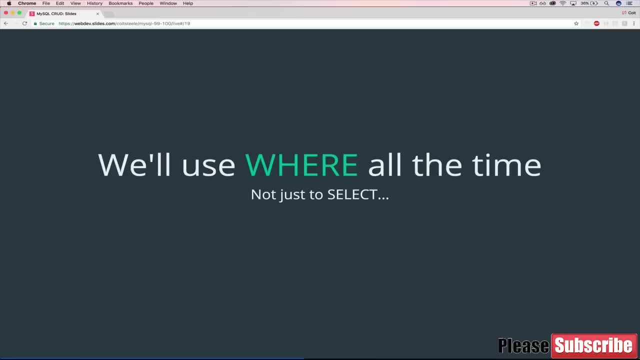 we will use WHERE all the time, So it's not just for searching or for selecting, But we'll need to use it when we're updating or deleting things as well, Because unless we're trying to update every single thing or delete every single thing, 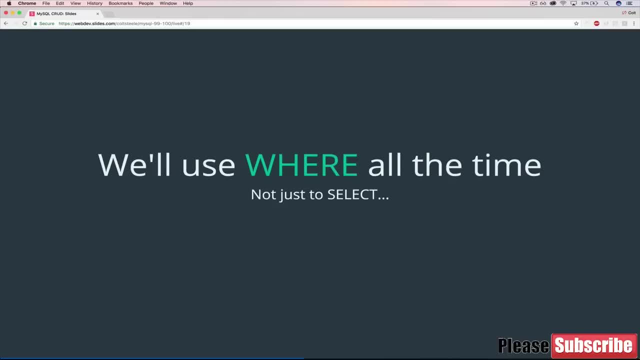 usually we want to update something specific. So we might say: I want to update the cats where their age is two and I want to make their age three Versus I want to update every single cat to have an age of three. 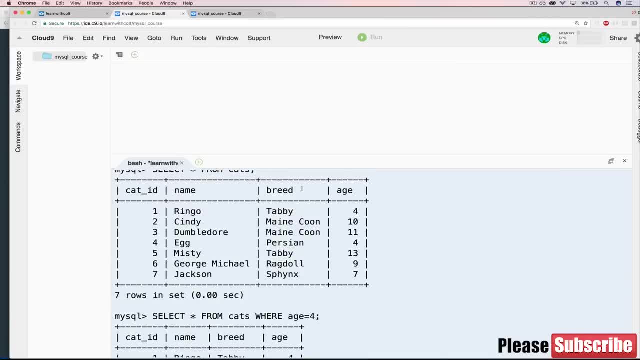 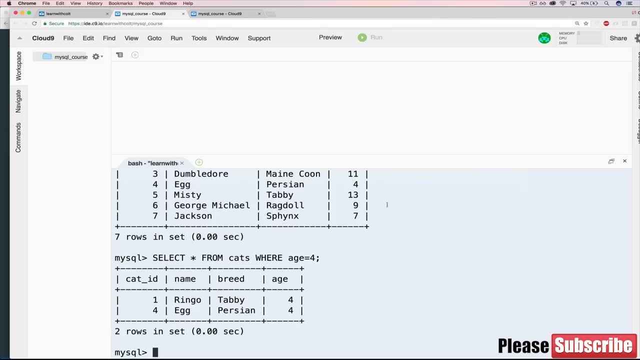 We could be more targeted using WHERE. So we're going to start by seeing how we use it to select. So here's an example: Select star from cats where age is four. So notice the syntax. here We have our same: select star from cats. 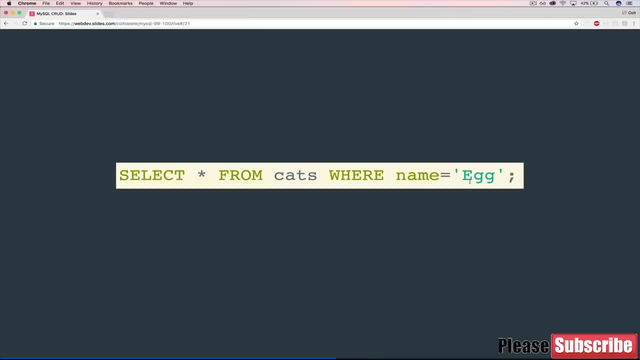 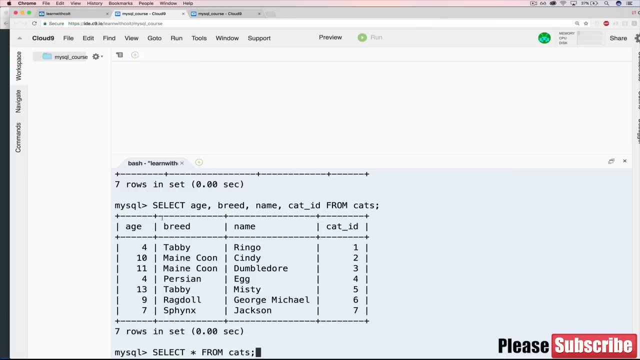 That will give us all cats. But then we have this WHERE age equals four. So what this will do is only select the data from the cats table where the age column is equal to four. And if we try that now, if we look at our data actually, 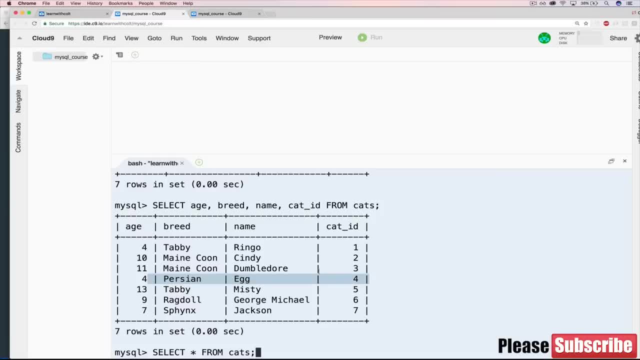 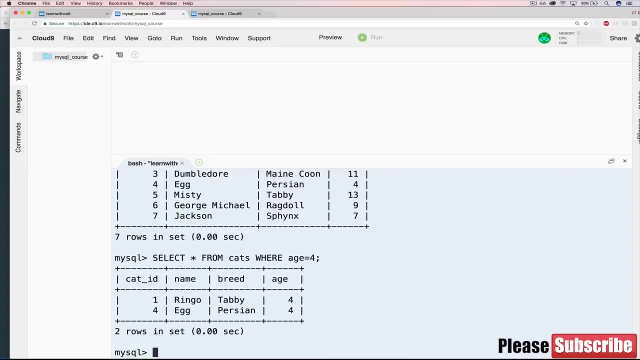 you'll see we have two cats, Ringo and Egg, who are both four years old. So if we do a select star from cats, you see what we get. But now if we modify that with our WHERE age equals four semicolon. 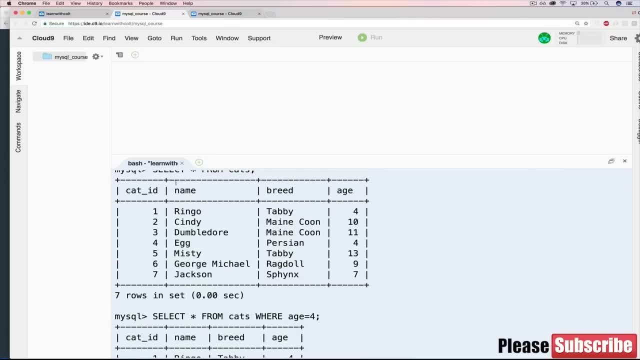 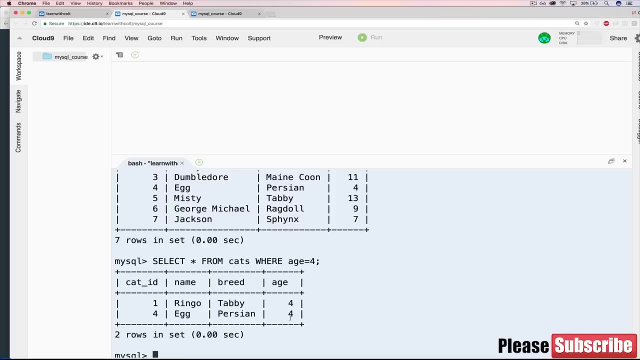 we only get those two results. So we still get cat ID name, breed and age because we used star, That tells us the columns, But now we only have two results because we used WHERE to get specific. One note: Notice that when I refer to age here, 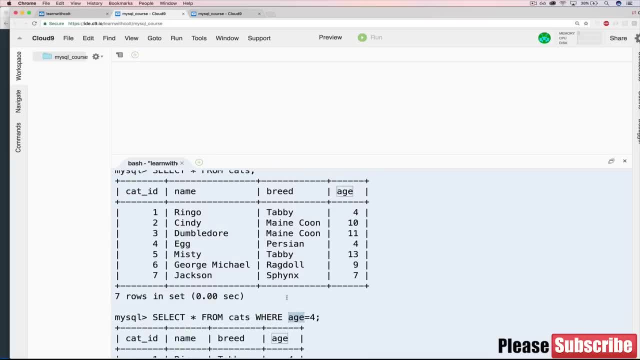 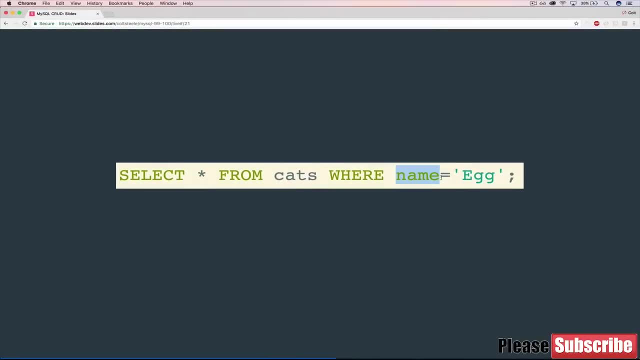 that is the column age, So there's no quotes around it. It's just age. So we can do the same thing here, but this time I'm using name to drill down or to get specific. So select star from cats where name is equal to egg. 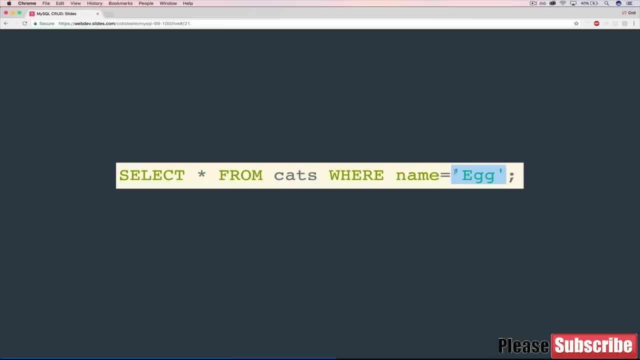 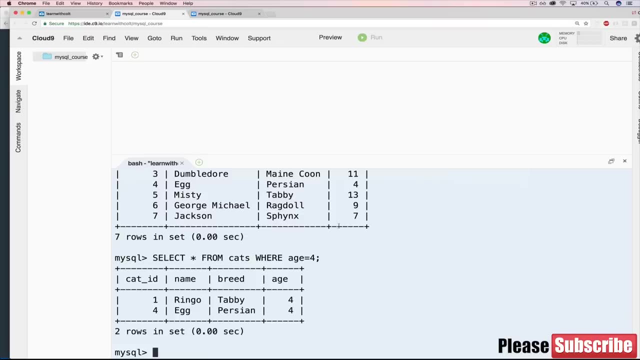 And notice I use quotes here because it's no longer an integer, Like ages, name is varchar, It's text, So we need those quotes. So we can try that now. Select star from cats where name equals egg, Just like that. 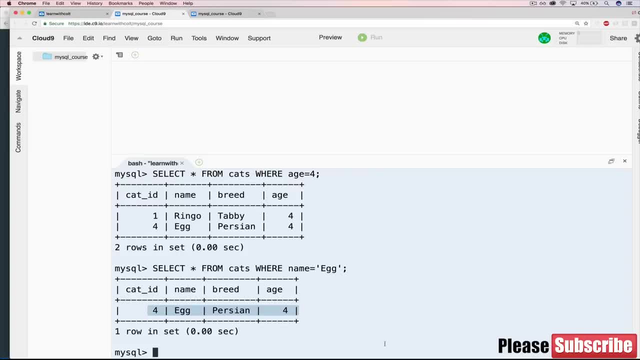 And you notice we get egg Cat ID name, breed and age. One side note while I'm here- You may come across this at some point: What do you think will happen if I fully capitalize egg? It still works. So it's important to note that. 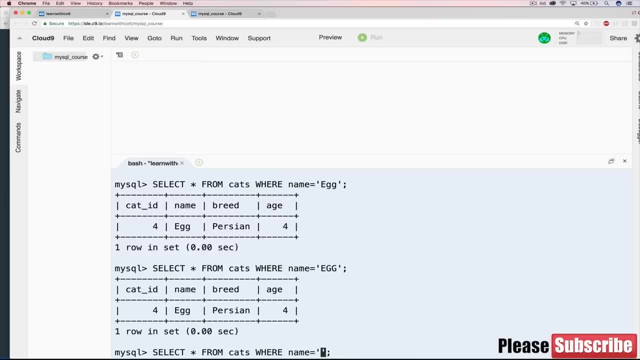 by default. this is case insensitive, So I could do lowercase g, uppercase G, And it still gives me the same data, So we'll see ways around this later on. Oftentimes it is useful, though, to not worry about case if you're dealing with things like 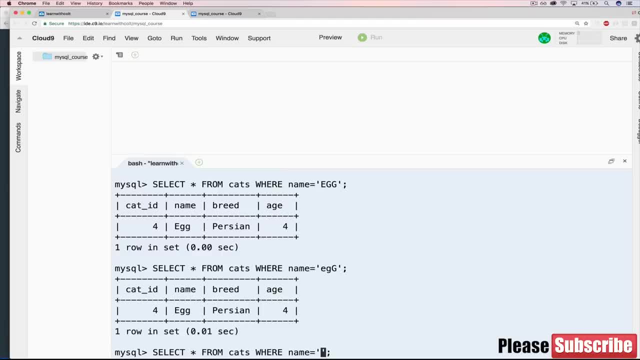 an email address where case doesn't actually matter. So if a user types in their email with a capital letter at the beginning versus lowercase, it should still be the same email in your database. But we'll talk about that later. I just wanted to point out that it's a thing. 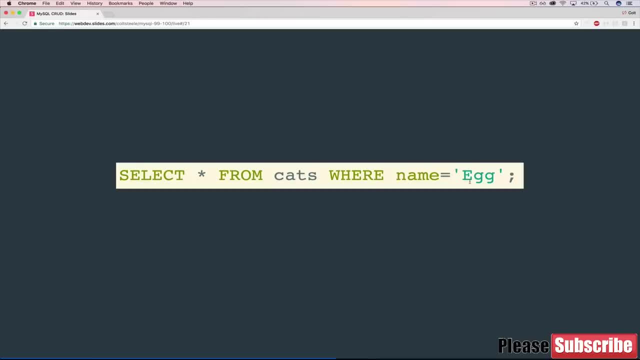 Case insensitivity. So that's all there is for now to the WHERE clause. Now there is a lot more that we will be seeing and working with. Like I mentioned at the beginning of this lesson, we will come back and use WHERE all the time. 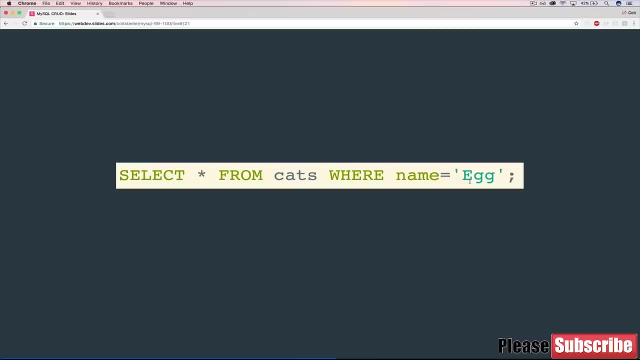 And in fact we're going to continue to use it for updating and deleting. Like I said, we need to specify what we want to delete and what we want to update. But I just want to make it clear we're not done with WHERE. 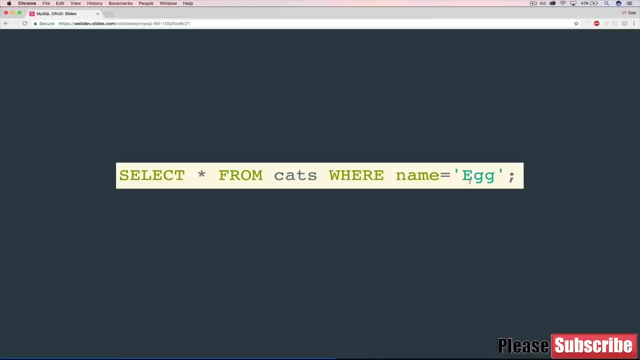 There's a lot of add-on functionality that we'll see in ensuing sections. Perfect, All right. So before we go any further, we have a couple of quick exercises that are just going to test you, basically on what we just learned: Select and WHERE. 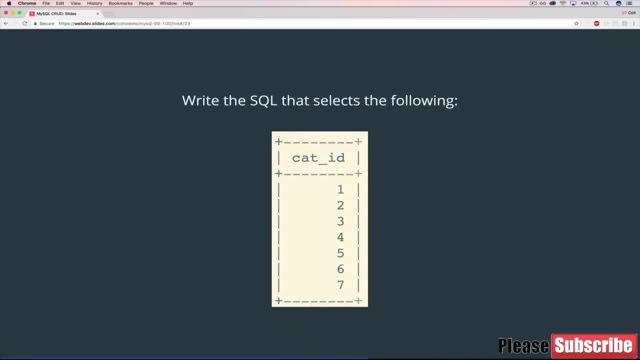 So the first one: I'd like you to write the SQL that will select the following: And this is using our cats, So the same data that we already had, which is why I asked you to- hopefully you inserted the same cats- Basically select all the cats. 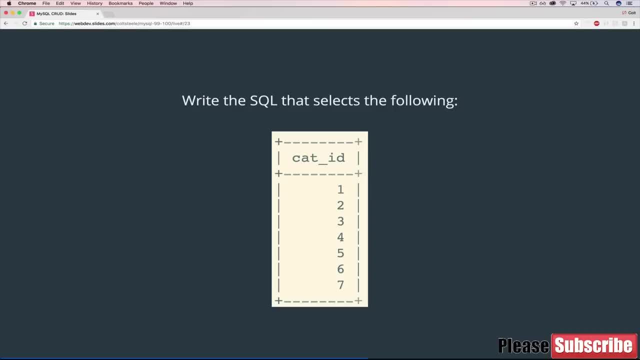 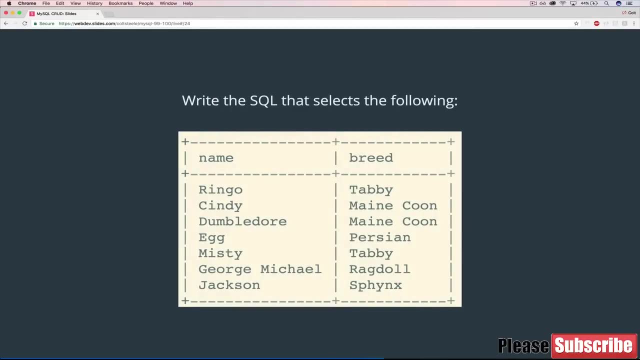 but only get their ID. And then the next thing I'd like you to do: of course, you can pause the video and do it and then move on when you're ready, to the next question, which is write the SQL that will select the following: 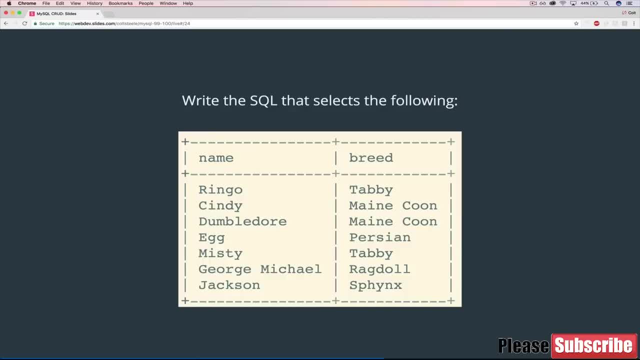 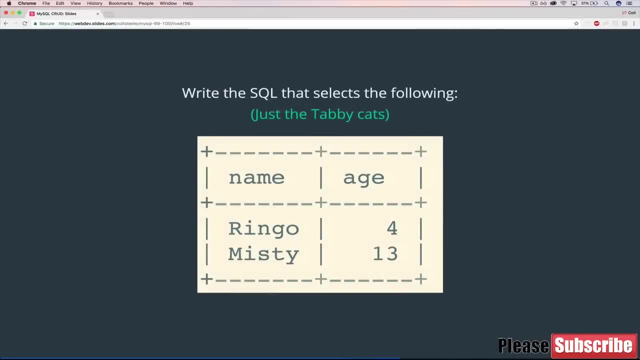 Name and breed only. So we don't want ID, We don't want age, Just name and breed. in that order for all of the cats. All right, And the next one is a little bit more complicated. You'll need to combine both things. we just learned. 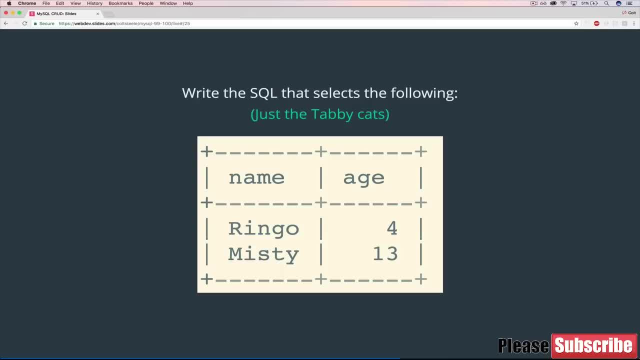 the SELECT expression and the WHERE clause. So in this case you're going to only select the tabby cats, So the cats that have breed equal to tabby, And we only want name and age. And then, finally, this is a little bit of a challenge. 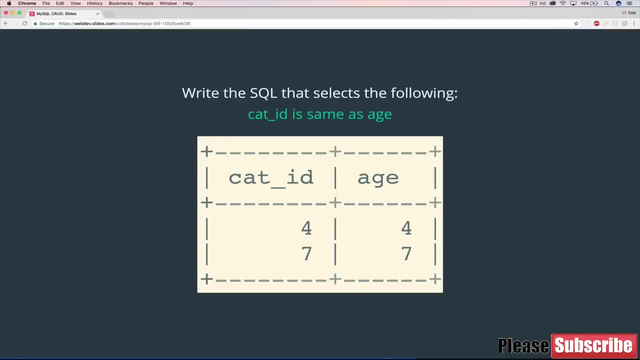 Because I didn't show exactly how to do this, But hopefully you'll be able to figure it out. We'll talk about it in the answer video either way, But hopefully it's not too difficult. In this case, what you're doing is selecting the instances. 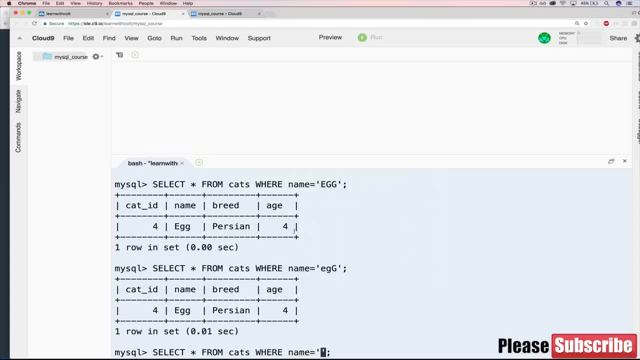 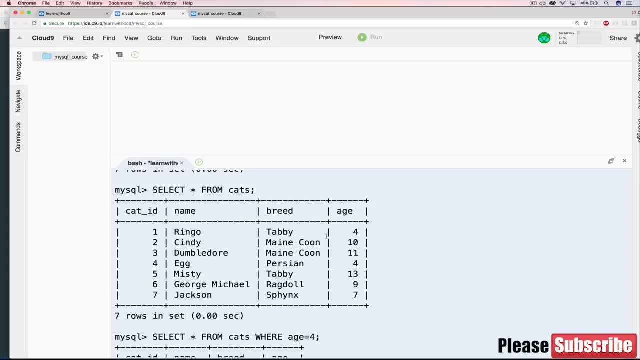 where cat ID and age are the same. So if I go back to the data here, when I select all of them, if you look here, cat ID and age they're not the same: 1 and 4,, 2 and 10.. 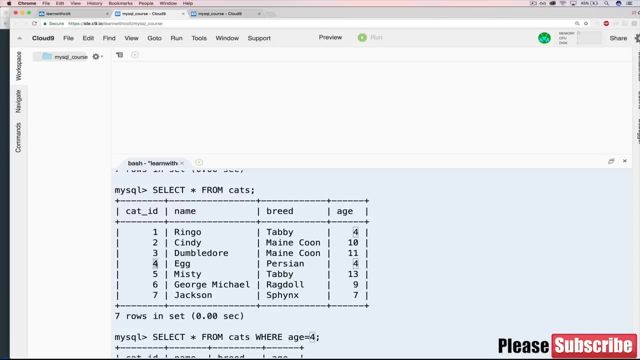 But egg cat ID is 4, cat ID is 4 and egg is 4 years old, And Jackson has an ID of 7 and is 7 years old. So how can you select just those two? And I don't want you to cheat. 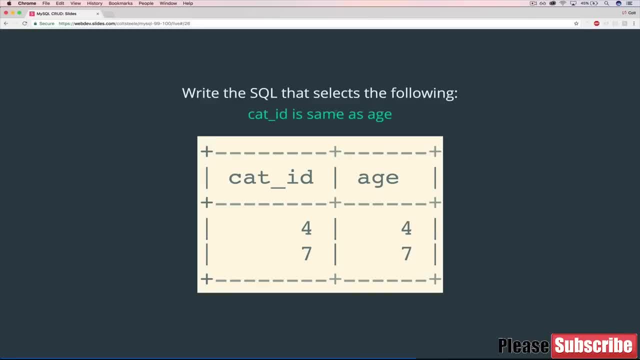 Don't select based off of their name or their breed or something. I want you to select where cat ID is the same as age, And we only want cat ID and age as well. Okay, solution video is coming up next, So let's see the answers here. 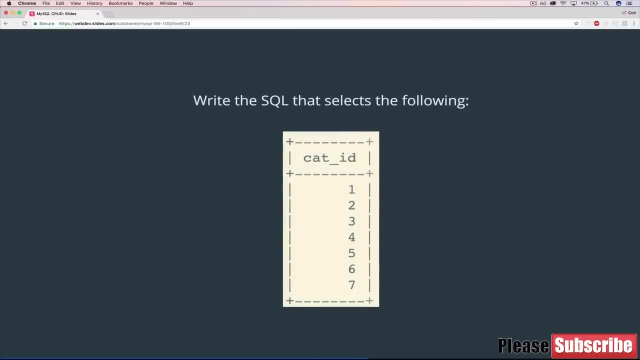 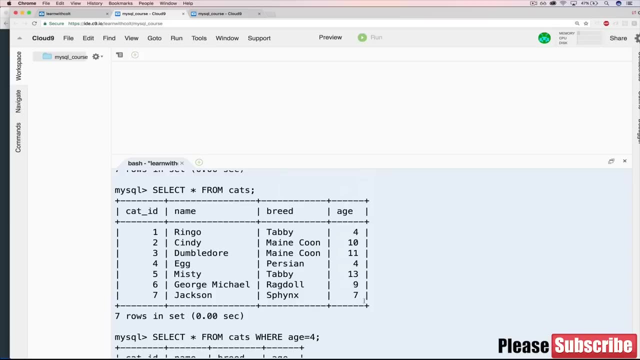 Feel free to skip forward if you feel like you got them right. So the first one: write the SQL that selects the following: We only want the cat IDs, but we want all of the results, all the cats. So that will be: select cat ID from cats. 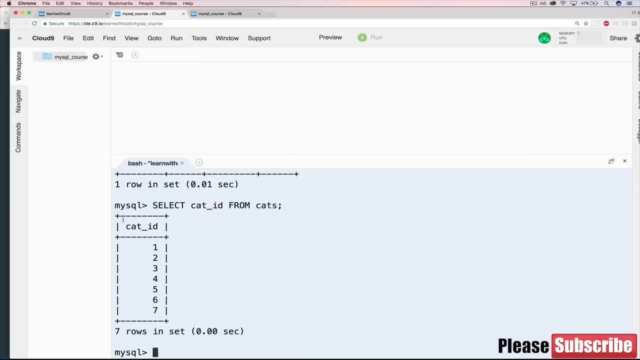 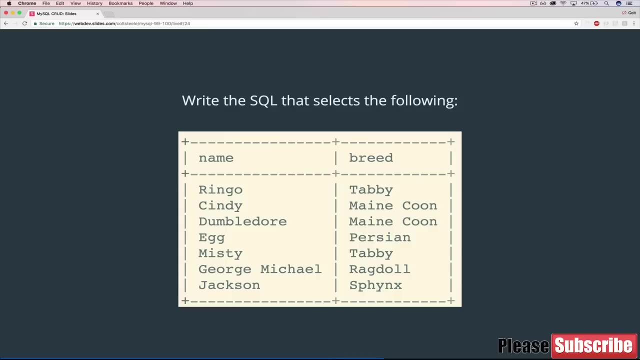 So we want all cats but only the cat ID returned, And that's what we get. Next up, write the SQL query that selects the following name and breed for all cats. So it's similar to the last one, except we want name and breed. 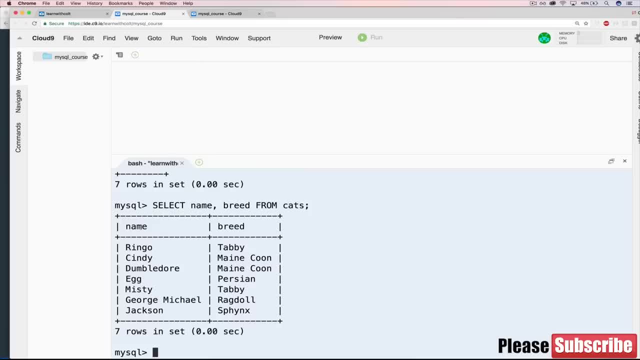 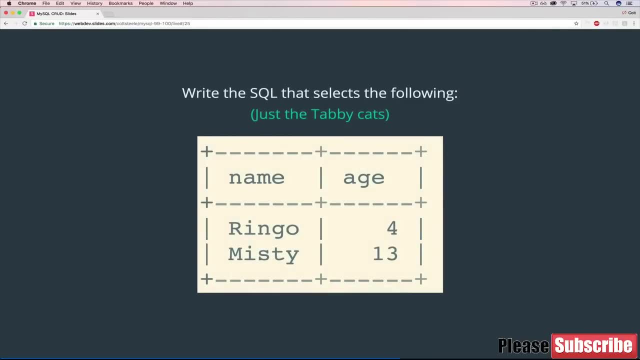 From all cats There we go: Name and breed, Okay. so let's talk about the solution to this one. here We need to use both the select expression and the where clause. We want to select name and age from cats where breed equals tabby. 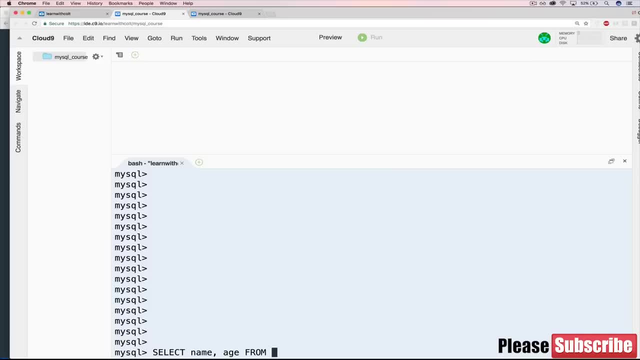 So let's do that: Select name, comma, age from cats where breed equals tabby, Just like that, And we get Ringo, who's four, and Misty, who is 13.. And that's exactly what we wanted to see. 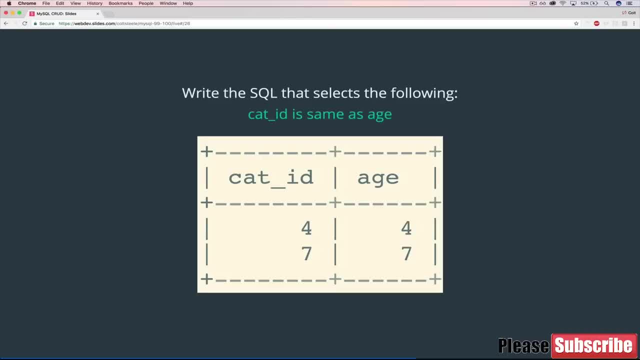 Now the final one is a little trickier. As I mentioned, we didn't see exactly how to do this, but hopefully you were able to figure it out because it's exactly the same syntax, but we're just checking a slightly different where clause. 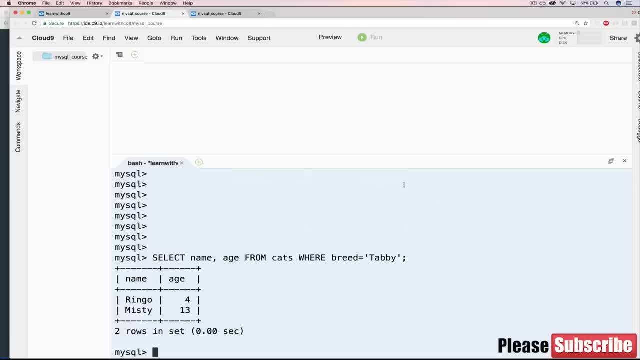 So we'll start with the first part. We want to select cat ID and age, So that's a select cat ID comma age from cats where- and we want where- cat ID is the same as age. So we've been doing things like where age equals two. 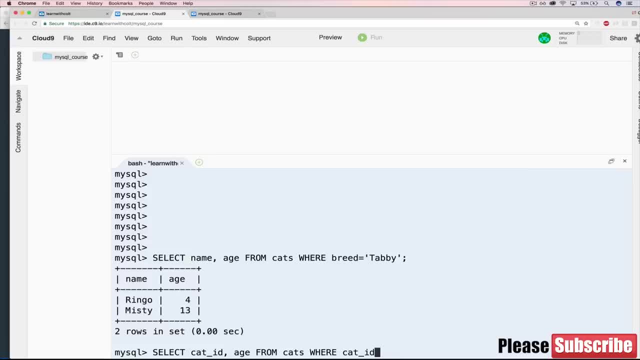 or we could do where cat ID equals one, but we can also just do where cat ID equals age. Those are both going to be numbers and MySQL is smart enough to figure that out, So it's going to compare cat ID and age and see where they're equal. 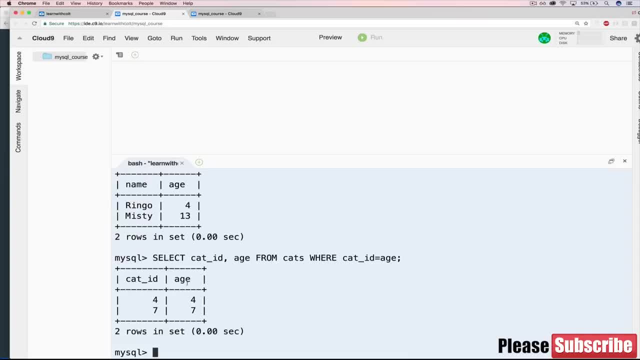 As you can see, we get what we want- cat ID and age- and they're equal. So let's go back and revise this a bit and do a select star, Just so you can see exactly what we're working with. We have egg in Jackson. 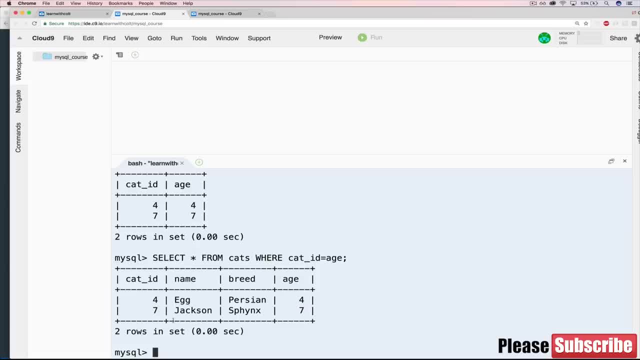 where age is four, ID is four, age is seven and ID is seven. Okay, So in addition to having some practice there, we also learned that you can compare columns and the values Rather than just picking an exact value like four or 10,. 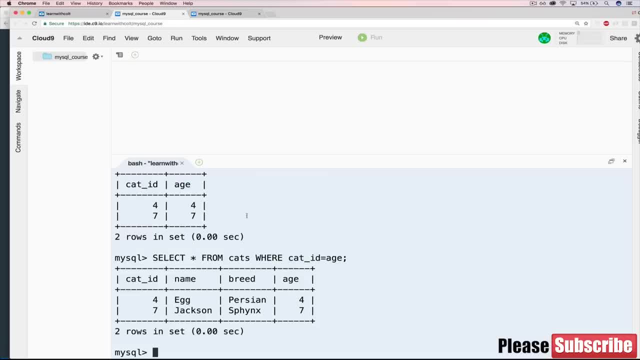 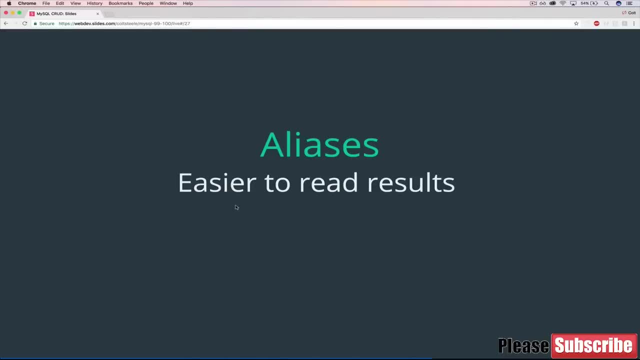 we can compare two different columns and select based off of when they're equal to another. All right, So one more thing we're going to talk about with reading data when we're talking about CRUD, Before we move on to updating and deleting. there's one other thing. 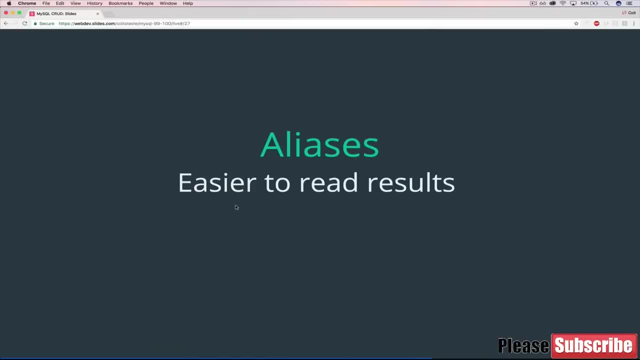 which are aliases. These are really simple, very short video. here. Basically, we can specify how our data should be displayed back to us. So what that means is, rather than having cat ID, name, breed and age here, I could tell MySQL that instead of breed, 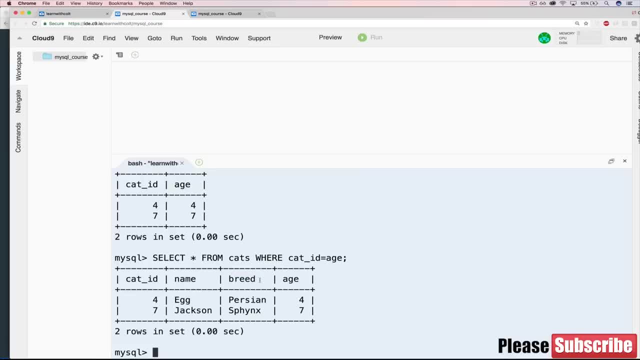 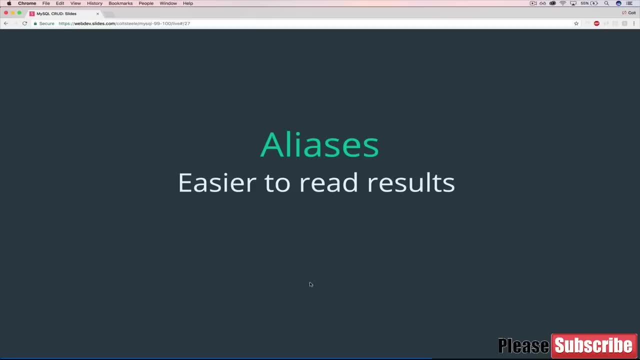 I want I don't know type of cat, Or instead of age I want years, And it won't alter the data itself, It just is how it's displayed to me. So let me show you a more specific example. Here we have, using an alias: 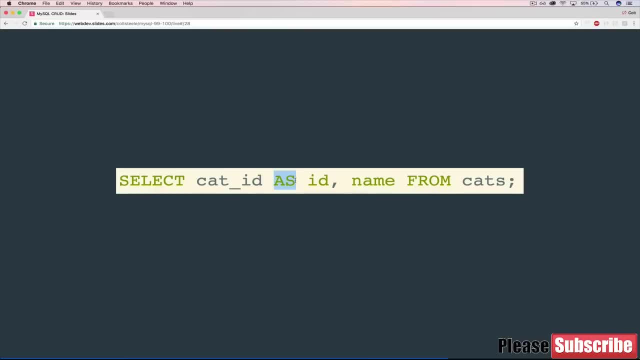 We're selecting the cat ID as ID. So rather than saying cat ID in the result it will only say ID And then name from cats. Now this is not that clear why it's useful And that won't become clear for a little bit. 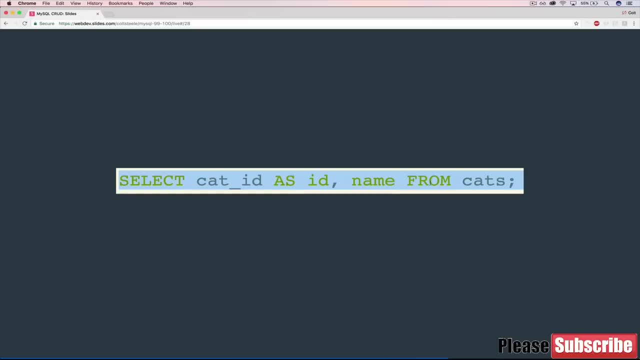 because right now our data is very simple and straightforward. But once we have multiple tables and we're selecting from, let me give you an example. Let's say we have a pet shelter where we have a cat's table and a dog's table. 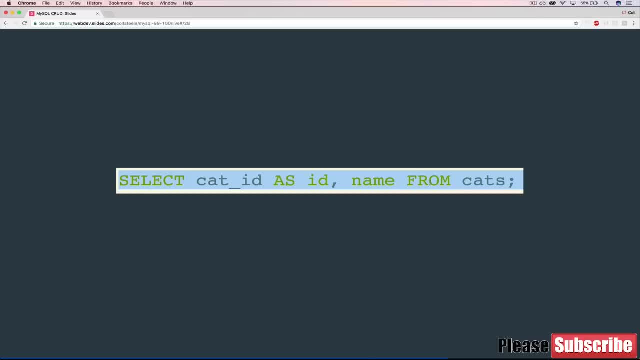 And both of them have a name. So dogs have names, cats have names, And when we talk about join tables- which you'll learn about in a little bit- that's when we take both tables and we select from them at once and combine them. 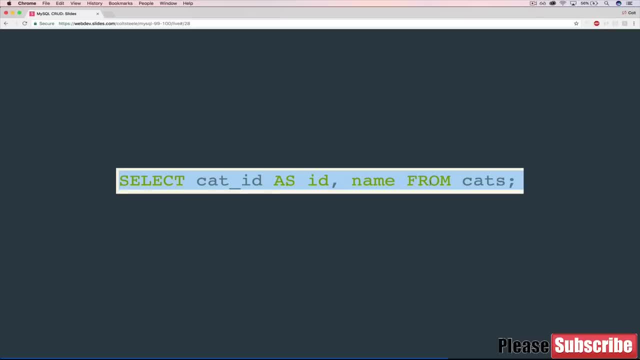 And the results. we would have two columns with name, So we would need to figure out which one is cat name, which one is dog name. So we could use this as to relabel it, So it wouldn't change the actual data. 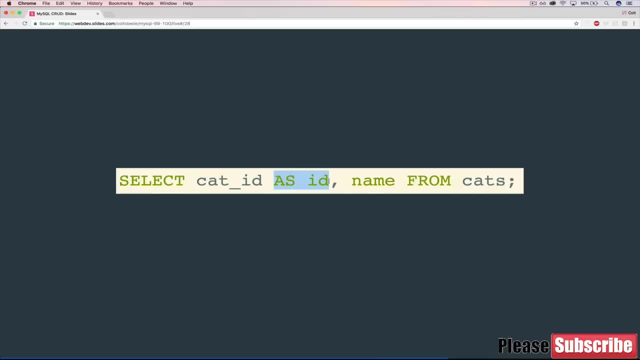 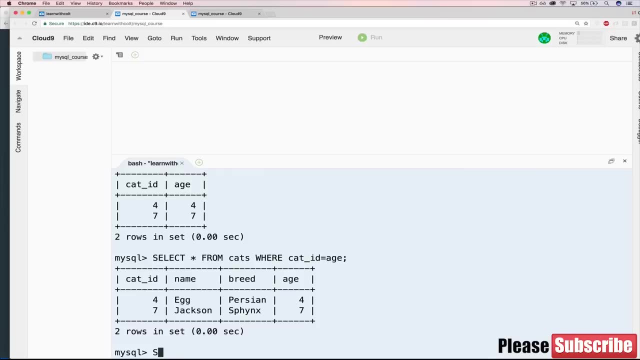 Our data is the same, The columns are the same, But when it's printed back out to us, when it spits out the data, it would use an alias. So if we try this now, cat ID as ID, common name from cats. 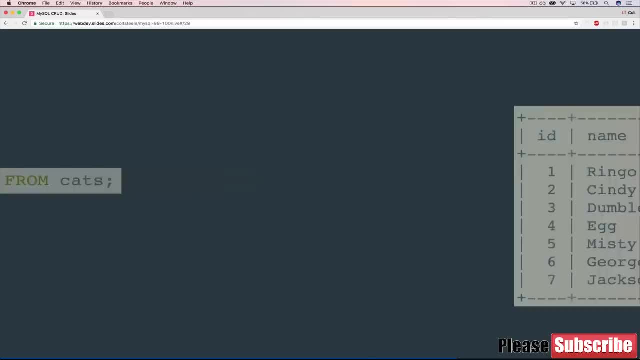 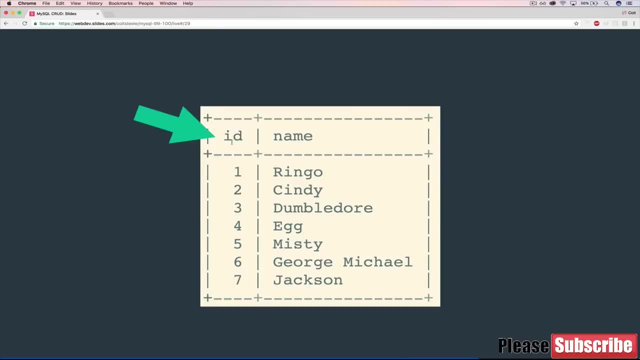 you'll see that we get ID here. And just to make that clear, I did the same thing And I even put a little arrow pointing to that ID. It doesn't say cat ID, It says ID. So also just to prove this: 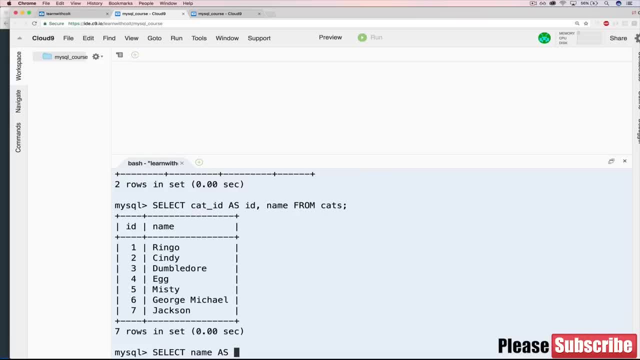 we could do something like select name as cat name, Or also, just to show you, we could use quotes to add spaces. So cat name like that comma. we'll also select breed as kitty breed- Why not From cats? And there you go. 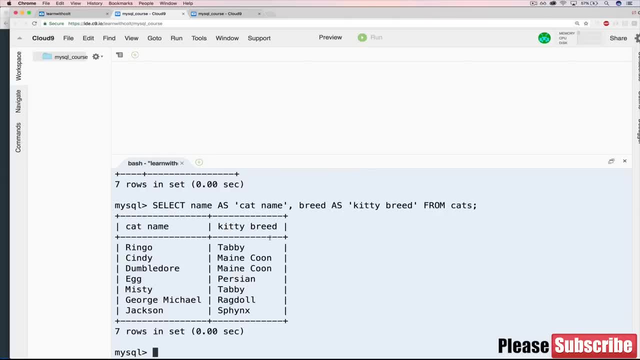 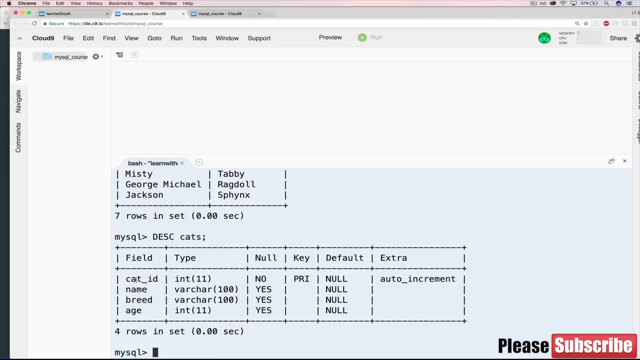 Our new column headers here are cat name and kitty breed, But of course, if we do a describe cats, you'll see nothing has changed. Our fields are still name and breed, Just when we print them out. So that's all there is to aliases. 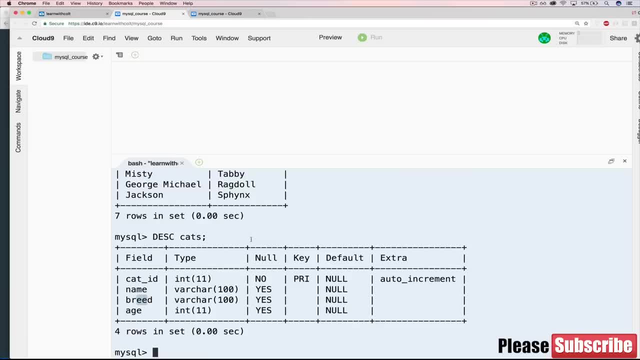 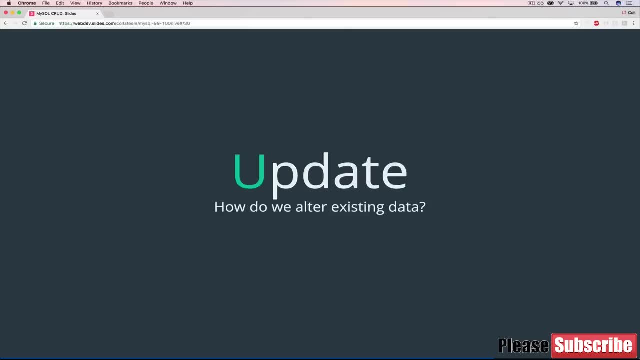 You'll see us using them later on, But I wanted to introduce them now so that you're not overwhelmed with a bunch of new stuff when we get to join tables. Alrighty, So we've covered the C and the R in CRUD. create and read. 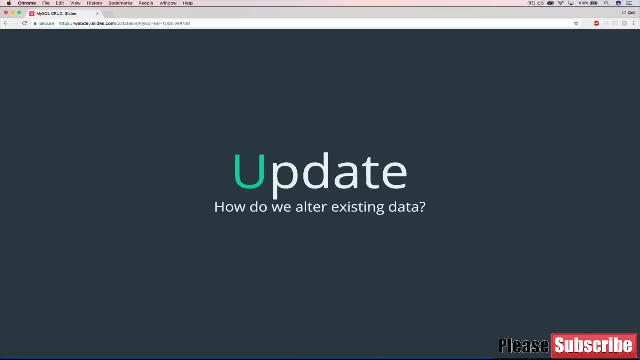 Now we're moving on to the U, which stands for update. So how do we update or alter existing data in our database? We've inserted something and maybe we made a mistake. We want to change it, But it's not always a mistake. 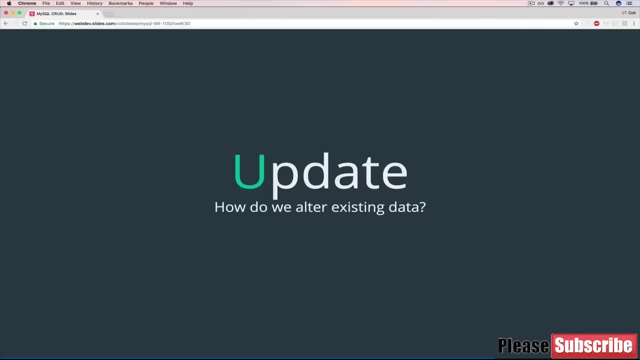 In our application. let's say we have users. Think about when you're updating your password. You forgot a password as a user, So you click the forget password link and you reset your password. Well, that needs to be changed in the database. 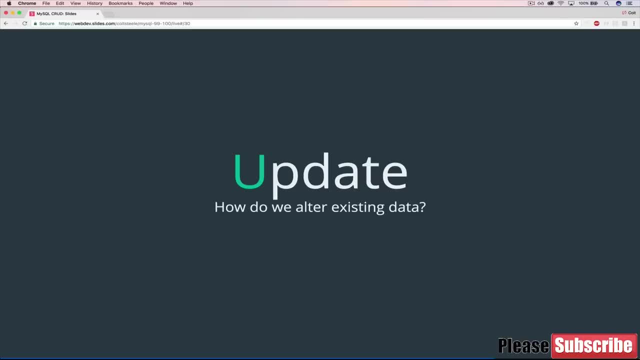 Or you change your profile picture on Facebook, Or you change your- I don't know- relationship status or something. All of that requires updating. So how do we do it? And the answer is that we use probably the longest SQL command you've seen so far. 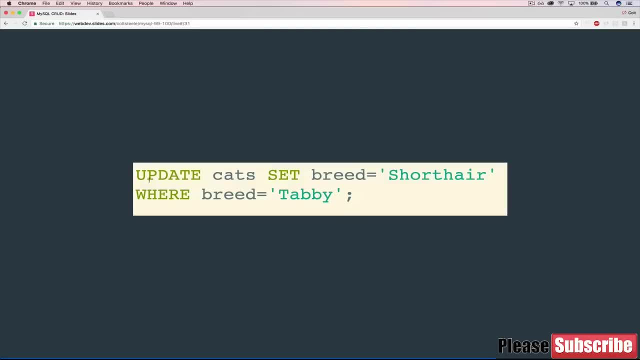 There's multiple parts, But the key words are update, set and where. So we've already seen where This is, where we tell MySQL which items in particular we want to select to update. So in this case, this entire line here is going to find: 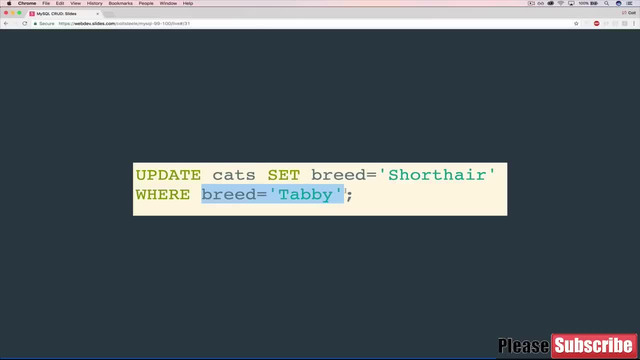 in the cats table all the cats who have a breed of Tabby And we're going to change that breed to be Shorthair. So again we have update and a table name Then set and this is a list of the changes. 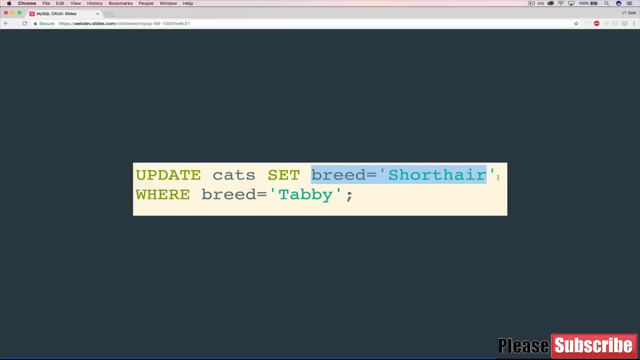 we want to make. So in this case, I'm setting the breed to be Shorthair. And then, who do we want to, or who is the wrong way of saying it? but what do we want to perform it on? What is the actual data? 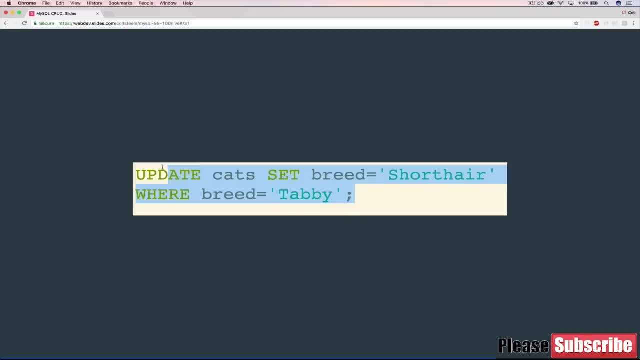 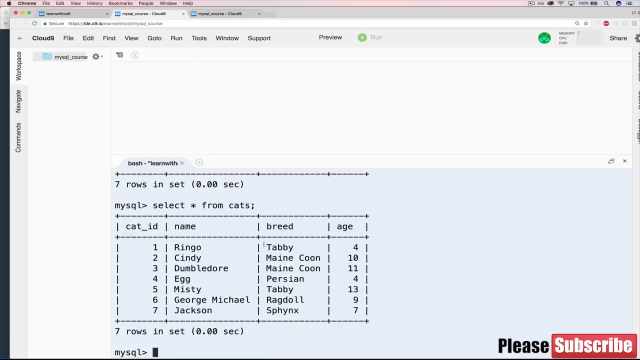 In this case, breed equals Tabby. So I will go ahead and just copy this line. Move over here, And if I do a select star from cats, you can see that we have two Tabby's right now: Ringo and Misty. 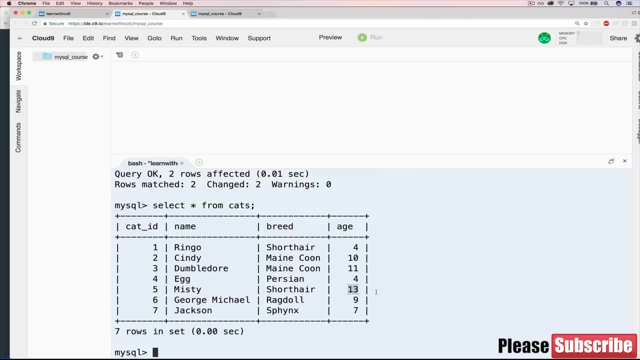 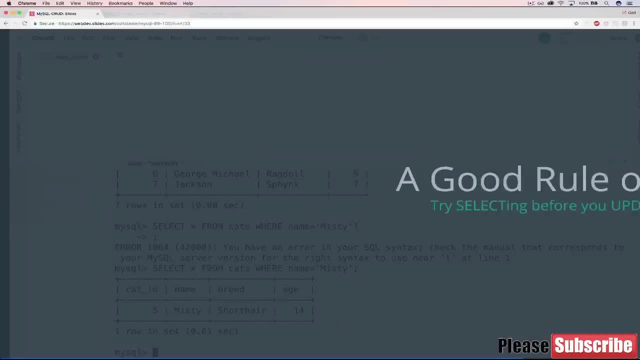 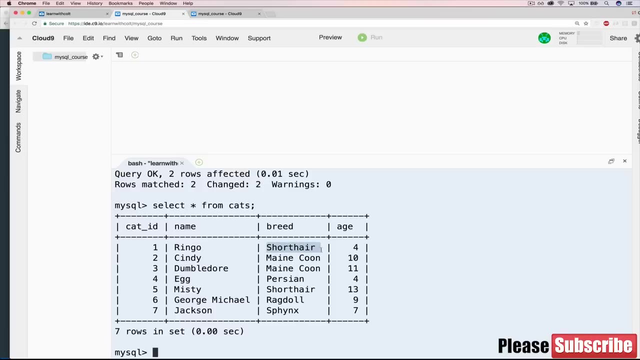 If I paste this line in update, cats change their breed to be Shorthair if their breed is Tabby. And now we select star again, You can see that both Tabby's, or previously Tabby's, are now Shorthairs. 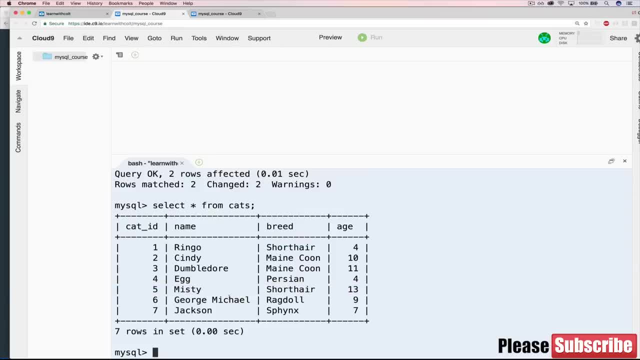 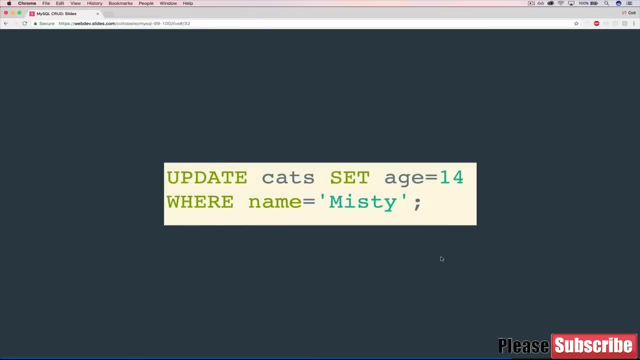 Misty and or, excuse me, Ringo and Misty. So here's another example. Let's say I wanted to change Misty's age to be 14. Right now Misty is 13. And we realize, I don't know. 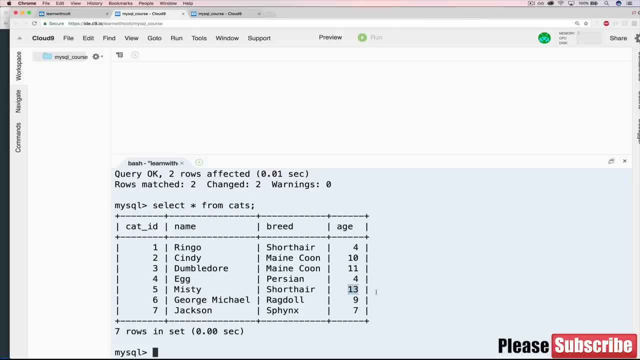 we realize that her dental records are wrong. Apparently, you can tell how old a cat is from their dental or from their teeth, So we misjudged how old she was and we want to make her 14 now. So to do that. 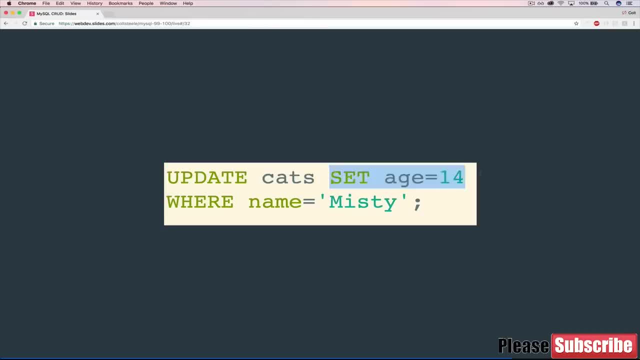 it looks like this Update: the cats table Set age to be 14.. We don't need quotes this time, because we're working with a number, an integer, And we only want to do that if name is Misty. So let's try it. 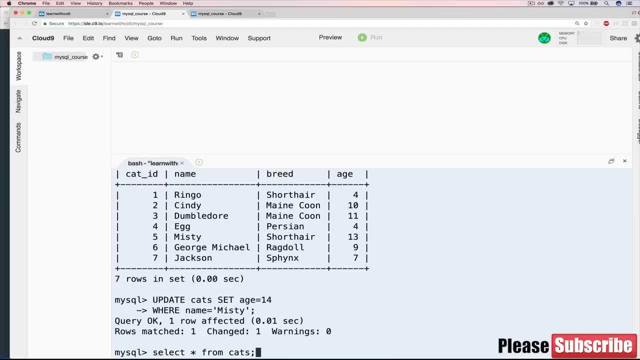 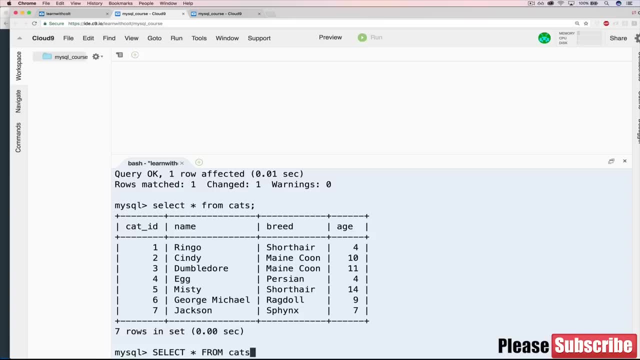 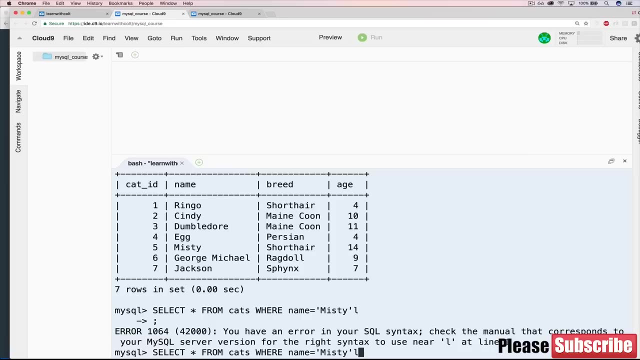 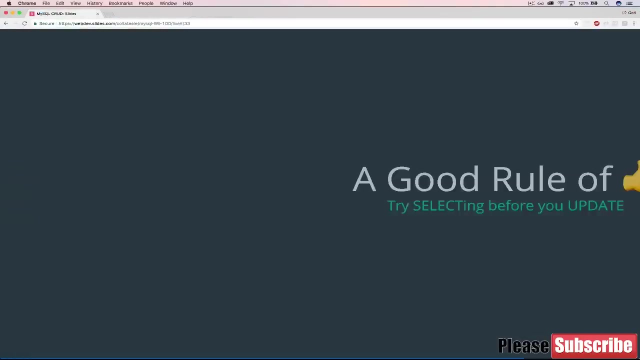 Now select star again. Or if we actually want to be more specific, we could do select star from cats where name equals Misty. Let's try that again without that extra L at the end. You can see Misty is now 14 rather than 13.. 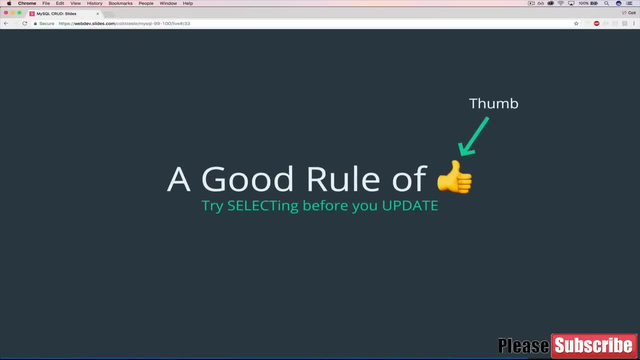 The last thing that I'll mention about updating is that there's a good rule of thumb that you should follow When you're updating something: you should make sure that you're targeting the right data before you actually do the update. So basically, run the select. 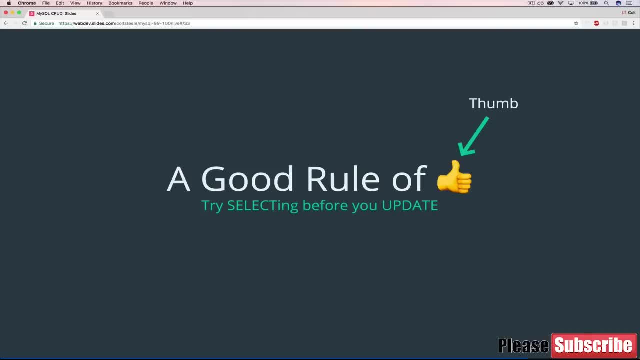 the equivalent select using your where query And once you make sure that returns the data you expect, then update it, Just so that you avoid accidentally updating the wrong data. And the same holds true when we talk about deleting, which we'll do in just a moment. 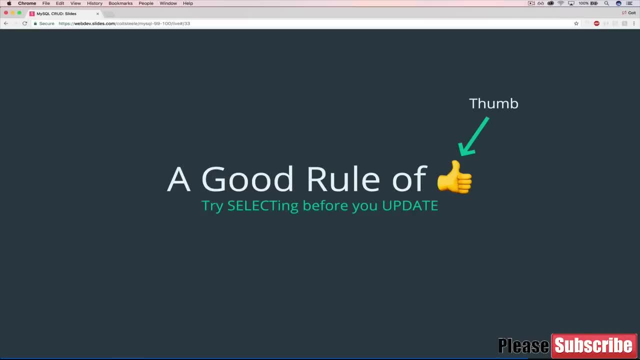 But the core idea is that there's no undo button So you could update something back manually if you messed it up. But you always want to just make sure you're targeting what you mean to target before you hit enter on your update. All right, so it's your turn. 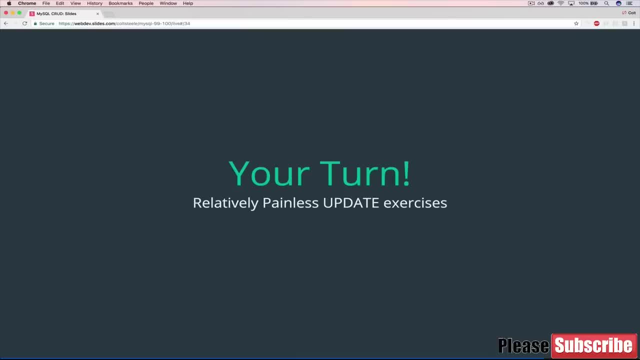 We have a couple of pretty painless- I hope- update exercises. They should be pretty quick. So the first one here is to change Jackson's name to Jack. Once you've done that, you can move on to the next one, which is to change Ringo's breed. 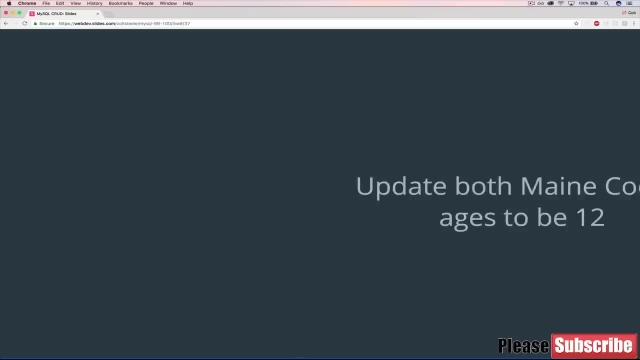 to British Shorthair And then finally update both Maine Coon's ages to be 12.. So there are two cats that have breed of Maine Coon. Make them both 12.. Okay, so in the next video we'll talk about answers. 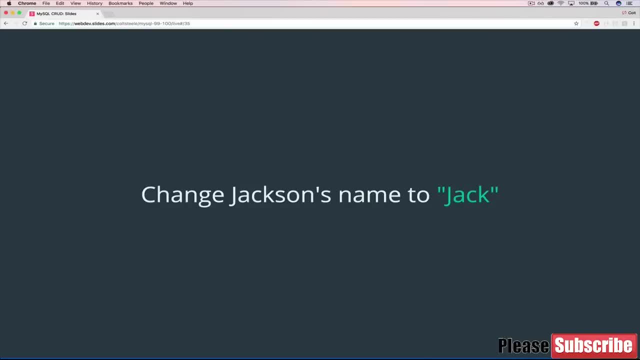 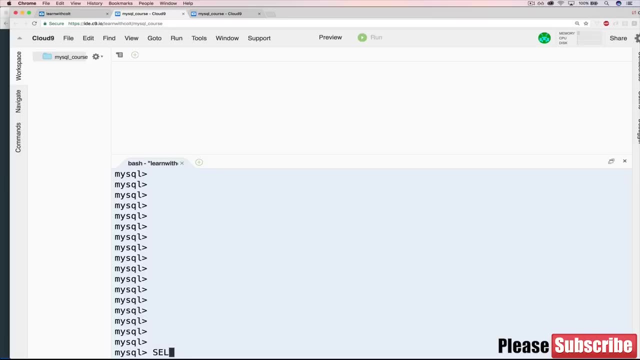 All right. So the first one is to change Jackson's name to Jack. So we'll practice what I just talked about: running a select before you do the update. So let's just try selecting star from cats where name equals Jackson. Okay, so we get Jackson. 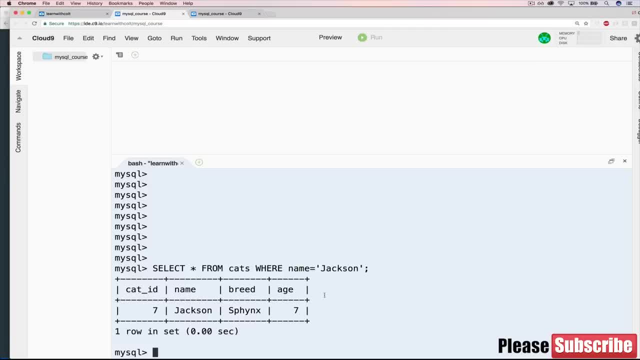 but we want to update his name to be Jack. So now we do our update: Cats set name equal to Jack. That's what we want to change it to And where do we want to change it? We want to change it where name is currently. 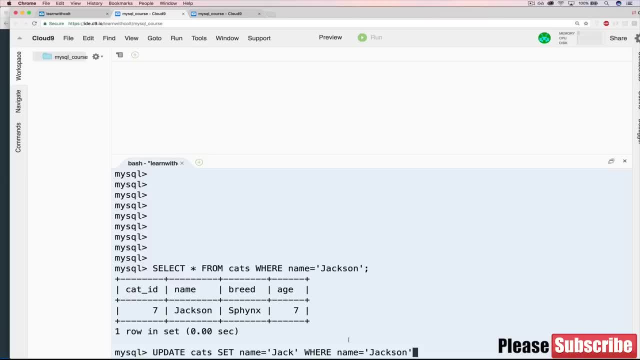 Jackson. Now I didn't specify that you had to use where name equals Jackson. You could also say where cat ID is 7 or where breed is Sphinx, because we only have one Sphinx right now. So any of those are valid Now if we do our select again. 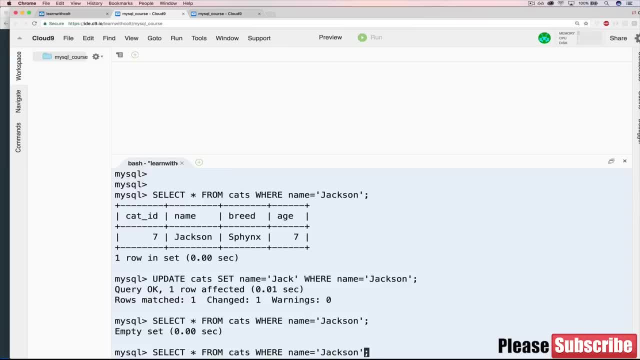 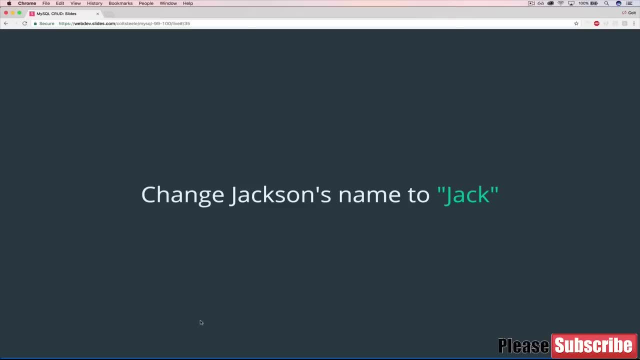 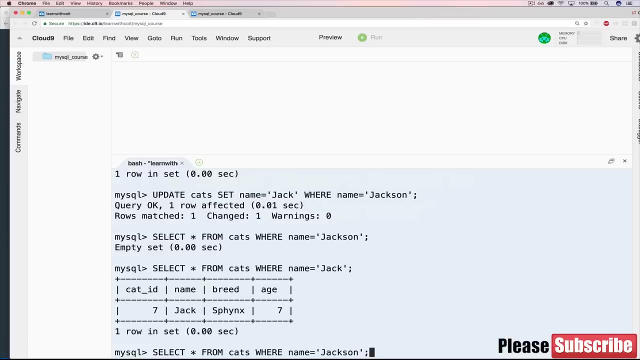 we get nothing because there is no cat named Jackson. If we change it to Jack, we get the same cat whose name is now Jack. Next up, change Ringo's breed to British Shorthair. So let's do the same thing, where we just do a select. 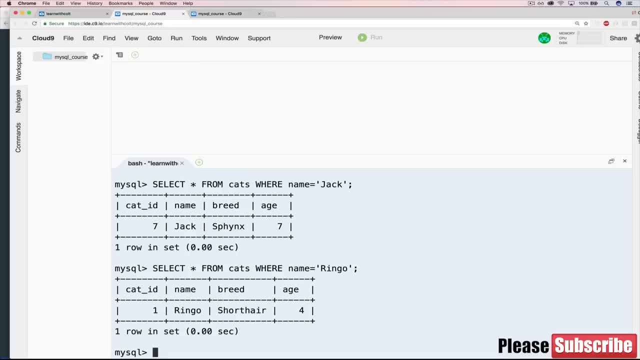 where name is Ringo. You can see that currently breed is Shorthair but we want to get more specific British Shorthair. So to do that, we do an update to cats set breed equal to British Shorthair, like that where name equals Ringo. 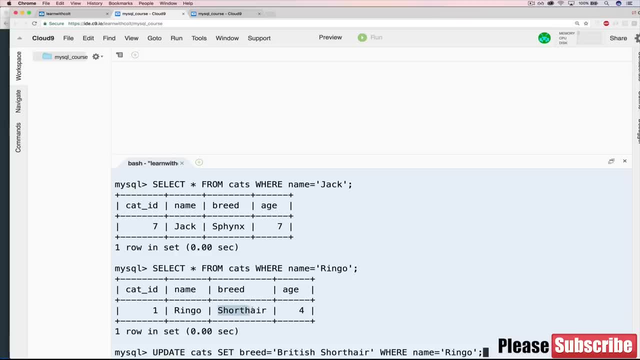 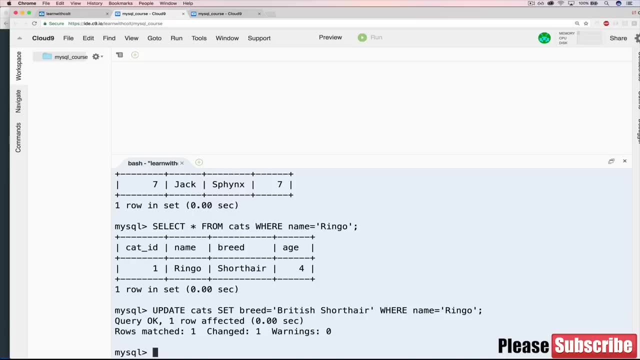 And again you could also do cat ID 1 or where breed is Shorthair. You could identify this cat however you'd like, But let's make sure it worked. So now, if I select where name is Ringo, we see breed is now British Shorthair. 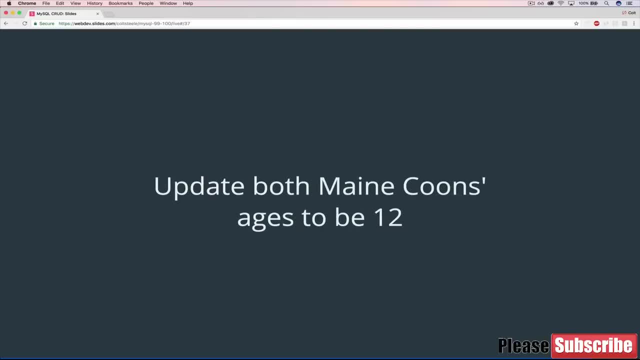 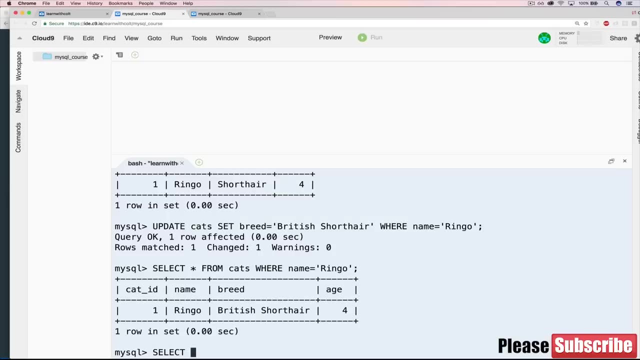 So the last one: update both Maine Coons, so breed equal Maine Coon and make their ages 12.. So let's just take a look at our current setup. in our database You can see we have these two Maine Coons. 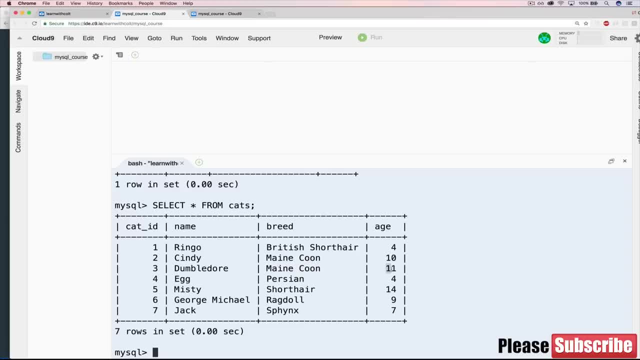 Cindy and Dumbledore. Cindy is 10, Dumbledore is 11.. For whatever reason, we want both of them to be 12.. So let's just select both of them. first. Select star from cats where breed equals Maine Coon, Just like that. 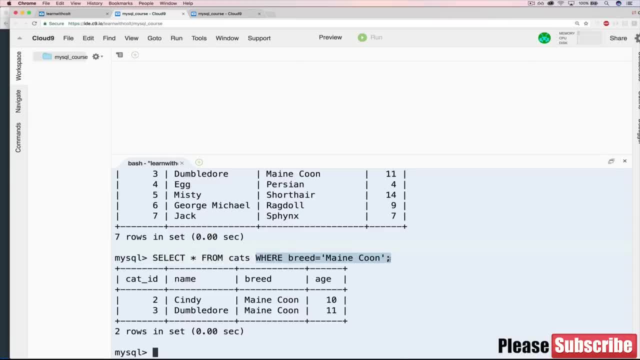 Perfect, So we are targeting them correctly. So we can copy that And then we'll do our update. cats set age equal to 12.. We don't need quotes Where, and I'll just paste that in And it updates both of them. 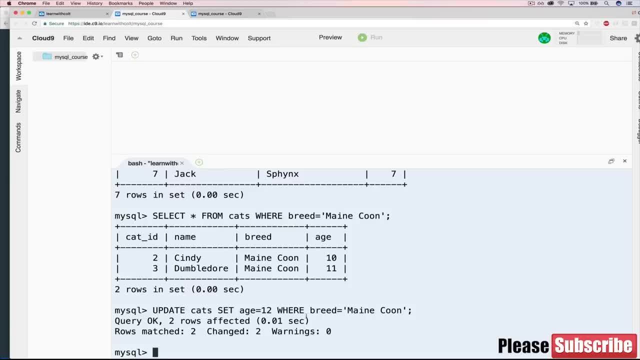 So that's really what I was testing here, is that you understood that where is not always just going to return one result: Whatever is returned will always be updated, which is also important to note that if you leave that where off- and I just said, update cats set age 12,. 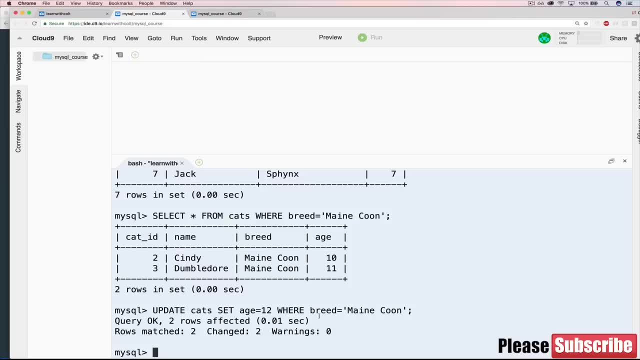 that would update every cat, which we don't want to do, which is why it's always important to select things first and make sure you know what you're targeting. Sometimes you might there could be reasons you wanted to update everything in a table. 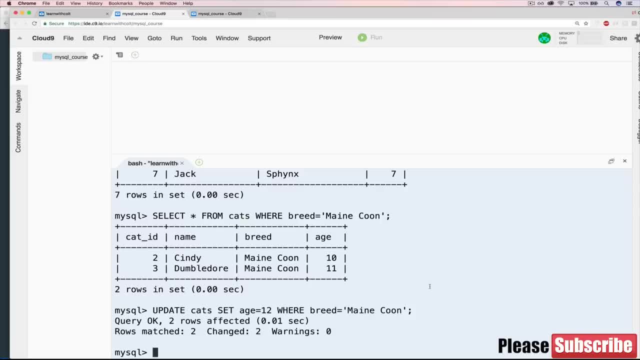 like if you were making a big change, or you are migrating something, or you realize that you made a big error early on in your application and you have every piece of data is wrong somehow maybe, but most of the time you're being very specific. 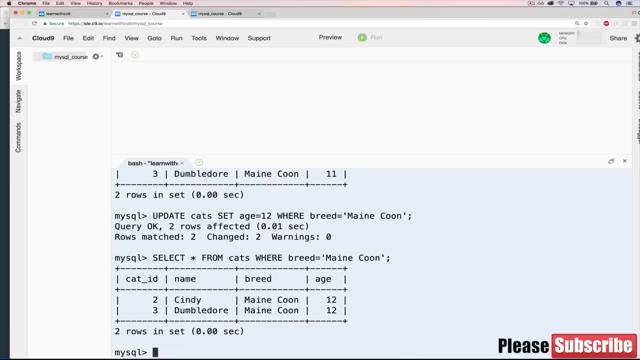 in the changes you're making. So just to double check: if we select again, you can see Cindy and Dumbledore are now both 12.. That's all you needed to do. Perfect. Next up, we're diving into delete. Okay. 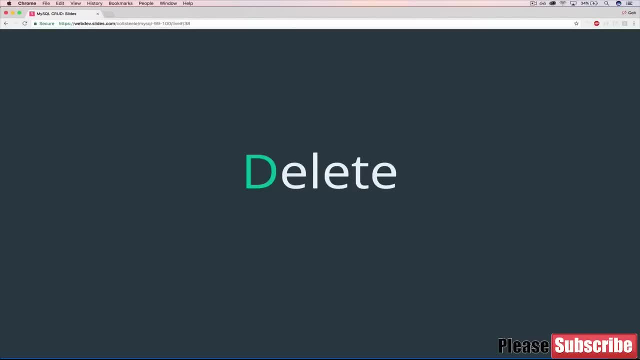 So we've made it through the C, R and U portions of CRUD. Now we finally made it to D, which stands for delete or destroy, depending on who you ask. So in this video we're going to see how to delete things in MySQL. 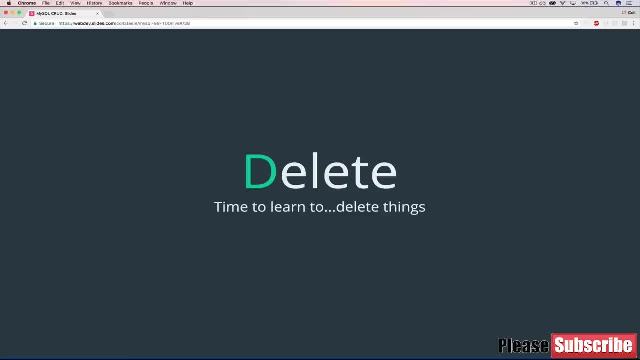 And it's pretty straightforward. It's very similar to selecting things, except, rather than just selecting something, you're going to delete it. So let me show you what I mean. So here's an example that will delete any cat with the name egg in our database. 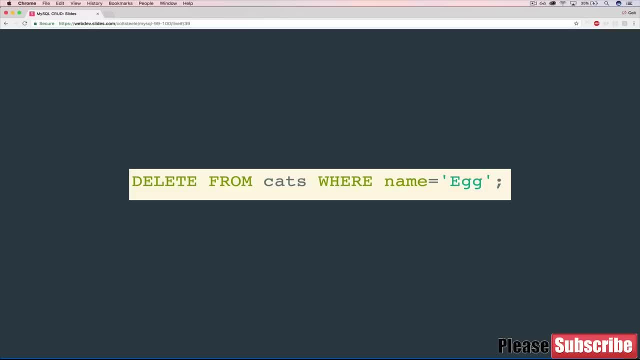 So imagine first of all that we were selecting. All we would have is select from cats where name is equal to egg. So if we ran that, it would give us the cat or cats with name egg and we can swap out select with delete. 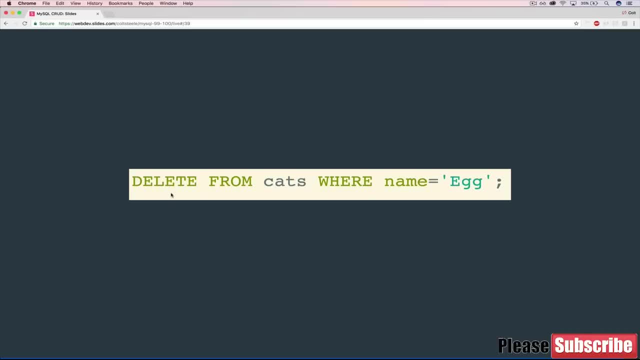 and that will delete it. So that same rule of thumb from before, where I said: make sure, before you update something, that your selection is correct. then do the update, because there's no undo button, unfortunately. Same holds true, and more so with delete. 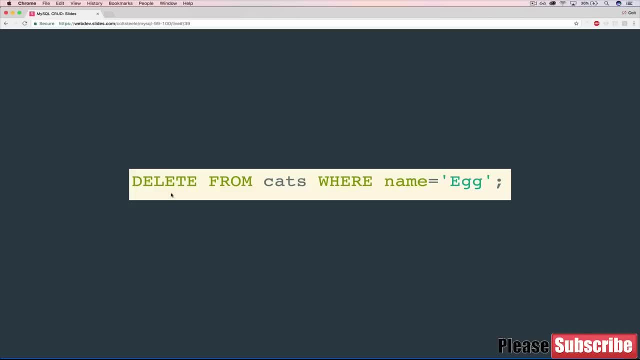 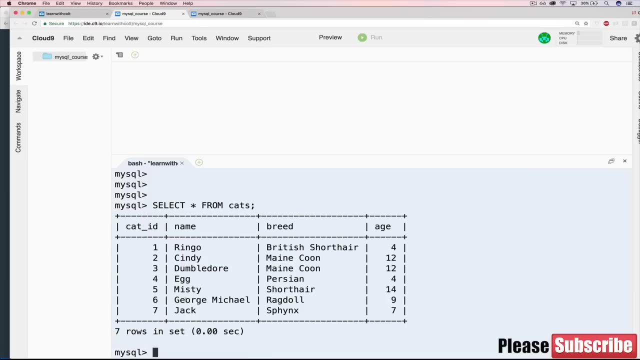 because your data's gone as soon as you delete it. So let's try this. We'll delete egg. Let's do first of all select star from cats. Just make sure we have egg in here. There he or she is. 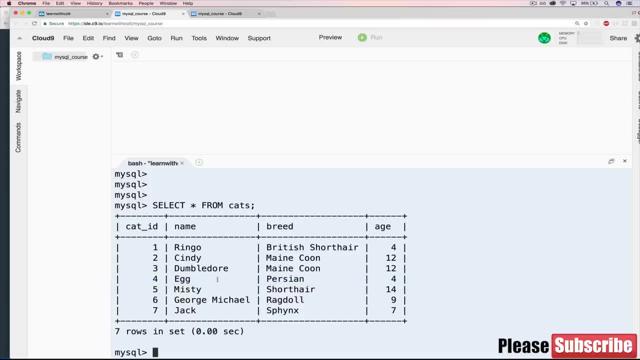 I'm not quite sure what I was intending with that name egg. So what we'll do first is just make sure we can select appropriately before we delete. So select star from cats where name equals egg. Remember that this is case insensitive, Just for now. 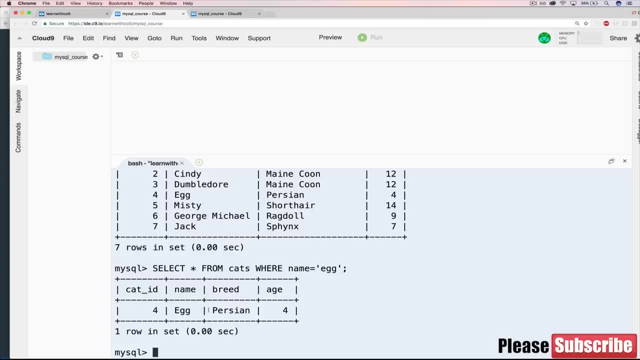 I'll do lowercase just to prove that. All right, so we get egg Perfect. So now to remove egg, delete from, and then we can just copy this. So before I hit enter, I do need to take a moment to address something pretty serious. 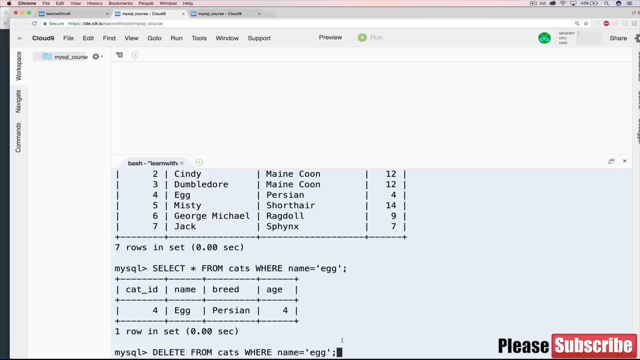 and that is that no cats are being harmed, No cats are dying here. Yes, they're being deleted from this table, but in reality, deletion doesn't mean death. It means that they're being adopted, perhaps to a loving family that will treat them. 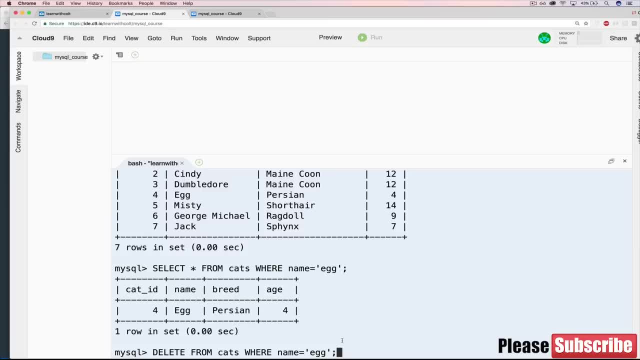 with the care that they deserve. So there's no death here and I hope I don't receive any furious comments about how I'm treating animals in my course. I love animals. I learned from my first course. I made a mistake. I will never refer. 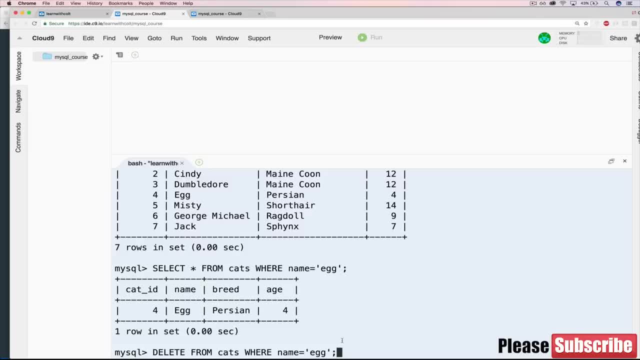 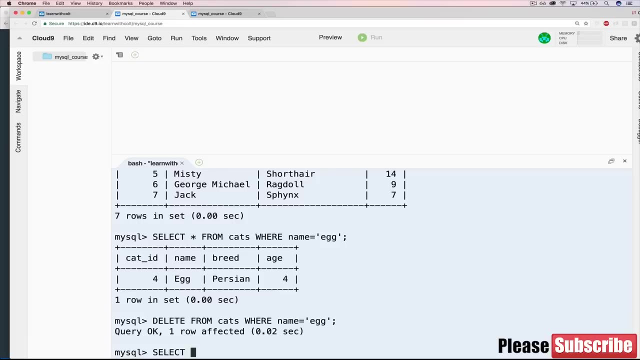 to deleting dogs or cats as killing them. I'm very sorry for that. So again, these cats are not dying. So with that out of the way, let's hit enter Now. let's go back and select star from cats and, as you can see, 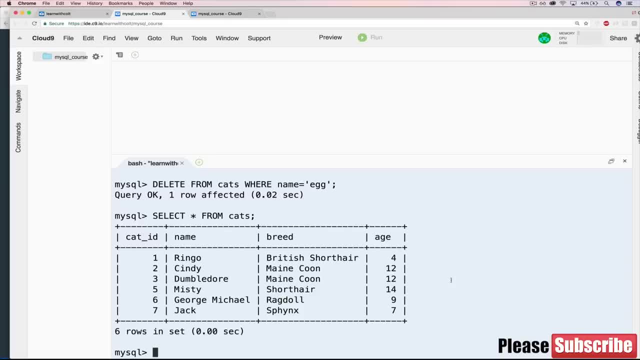 egg is now gone- Also something that does come up sometimes. notice that the cat IDs have not shifted. They're still the same. Some of my students in the past have had the expectation that the IDs would alter, but they always will stay the same. 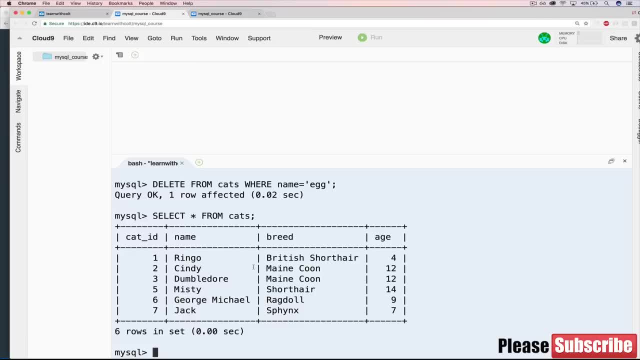 And that's because when something is inserted into a table, that unique ID is generated for it. Remember, it's a primary key And eventually we'll learn about having multiple tables that interact with one another and we'll be storing these IDs. 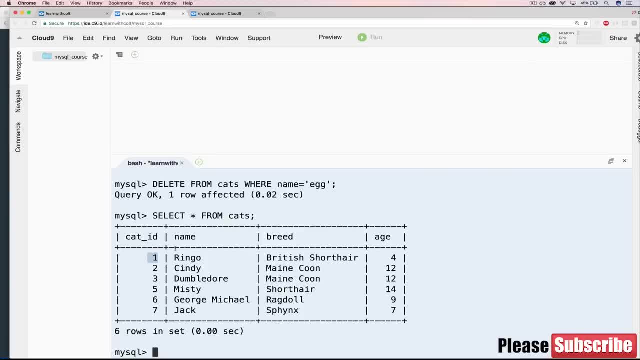 in other tables. So if it changed, that could be problematic because we'd have to change it in multiple places. Anyways, all I'm trying to say is that we removed four, but we still have five, six and seven. This didn't change to four. 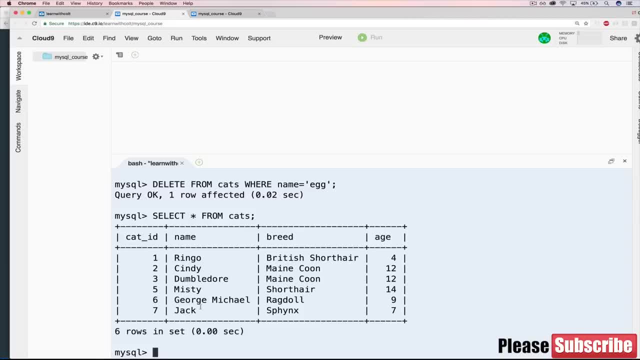 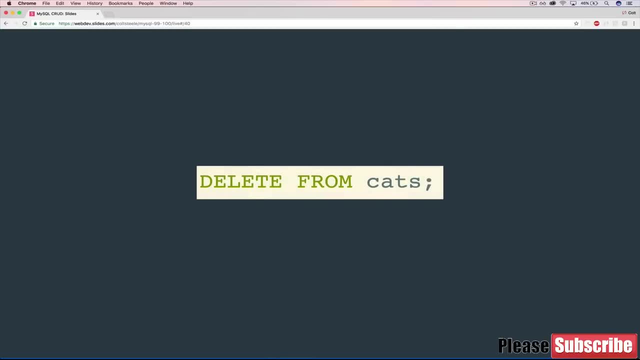 this didn't change to five and so on. All right, So we deleted that Rest in pe I mean: enjoy your new life with your happy family egg. So one last thing here is that if you look at what I've written here, 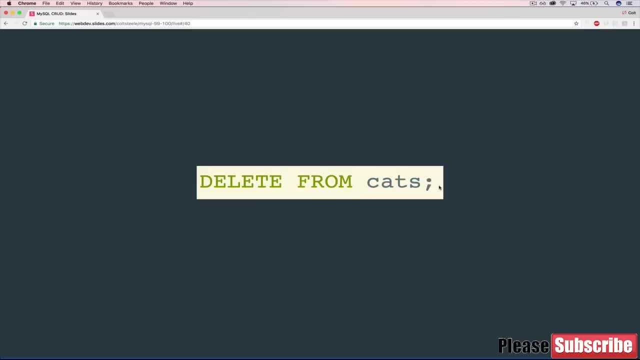 delete from cats. what do you think that will do? Now, I don't run it, but what do you think this would do? And the answer is that it deletes everything, all cats. They're all released to their happy families. So that's important to know. 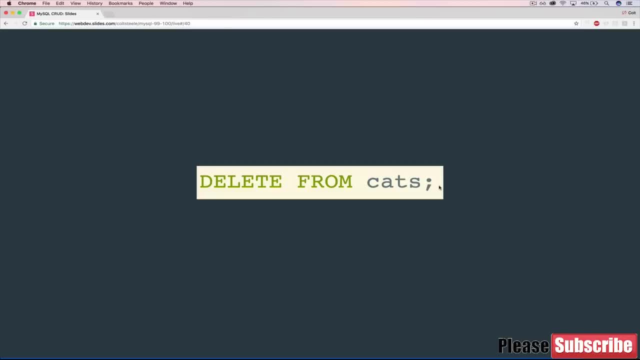 that you can do that. So it's different than dropping a table, because dropping a table gets rid of the table entirely and all data inside of it, But deleting from cats just deletes the entries in the cats table, but we still have the shell. 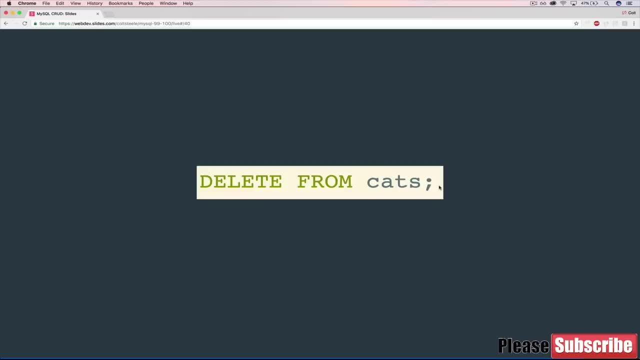 We still have the cats table. There shouldn't be very many times when you need to use this command. I'm not going to do it just yet because I want us to have our cats data for a little bit for the next exercises, But just keep that in mind. 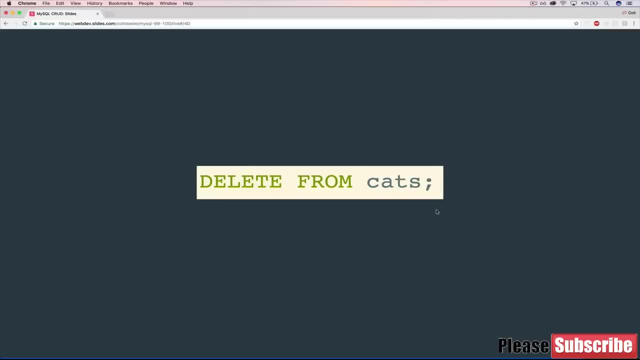 Because we didn't specify a where clause over here. it's the same as selecting without a where clause: It selects everything, So this will delete everything. Okay, Next up, you're going to practice deleting. All right, So it's your turn here. 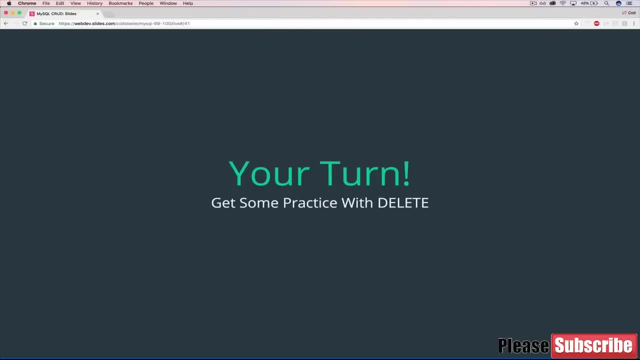 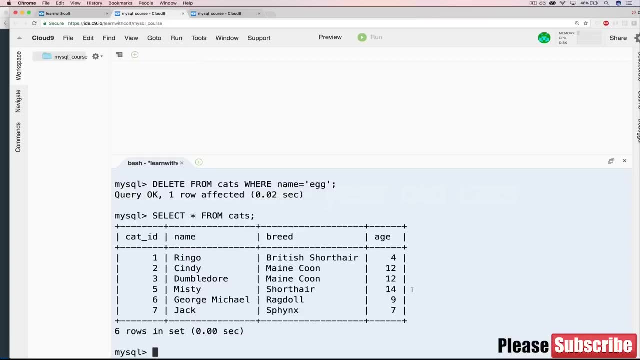 We're going to get some practice with delete, So we have three different things I'd like you to do. The first one is to delete all cats that are four years old. So if we look at our data, there's only one right now. 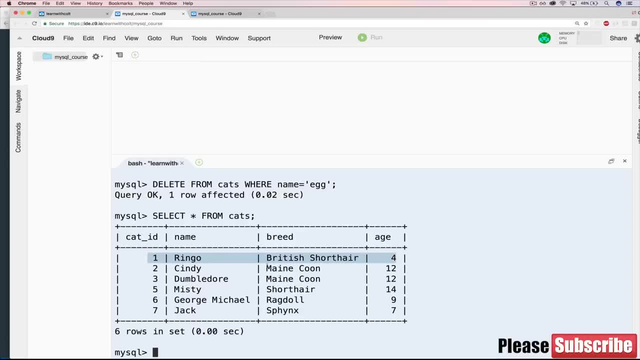 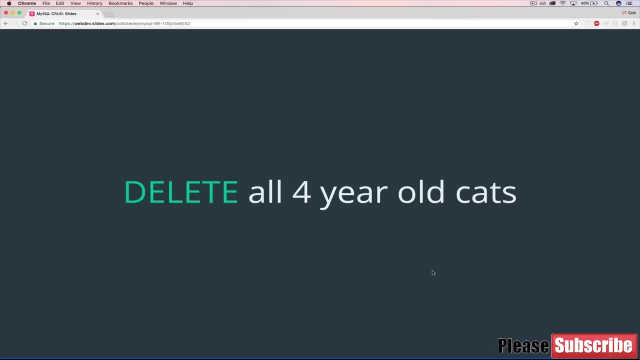 because we got rid of egg. But I would like you so don't just say delete Ringo or where breed is British Shorthair or ID is one, but use age. Then the next is to delete cats whose age is the same as their cat ID. 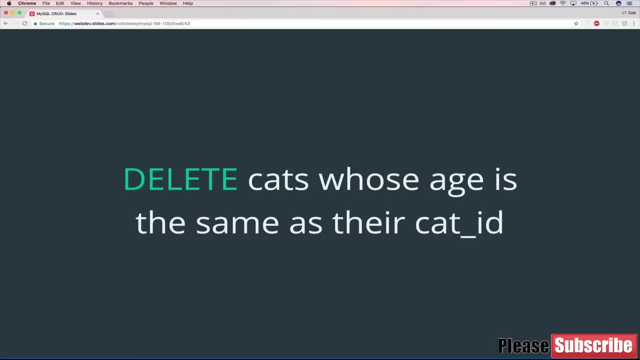 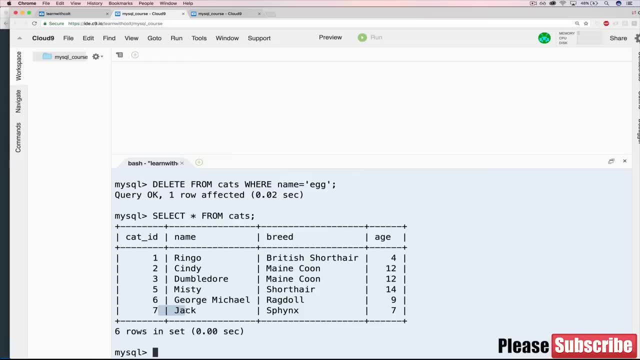 Now I had to do something similar to this with the select exercises. Now you'll need to put that together with delete. So in our case, it's only Jack at this point. So Jack has an ID of seven and age of seven, But once again, 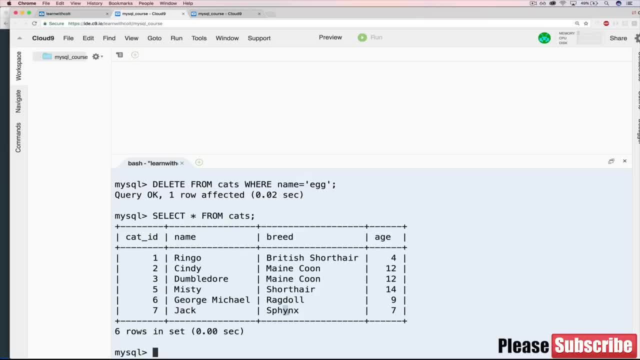 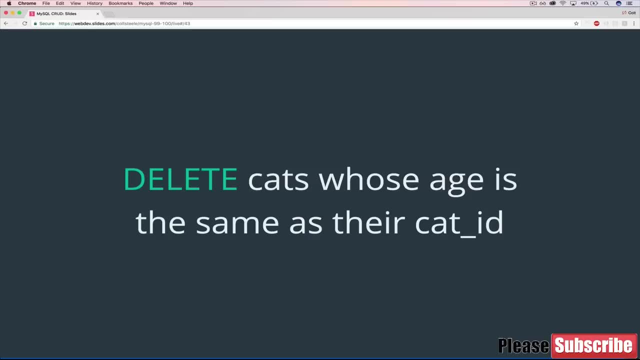 no cheating. Don't just select based off of name or breed. Do it the way I specified, please. I mean, it's up to you, but the way I recommend. Next up is to- oh my gosh, delete all cats. 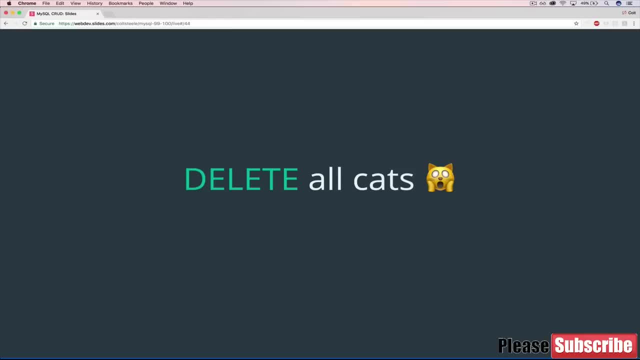 So that thing that I said I wasn't going to do because I didn't want to delete all of our data, Well, you're going to do it, And then we'll be starting with a whole bunch of new data in the next exercise. 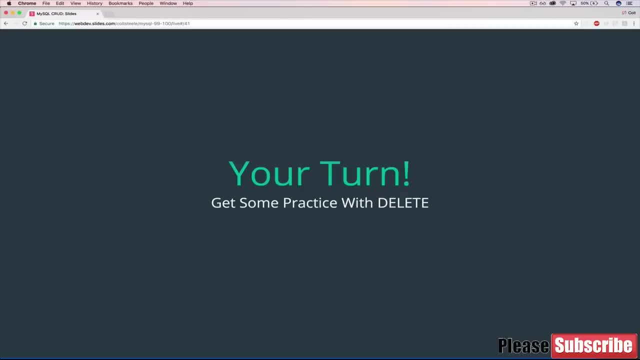 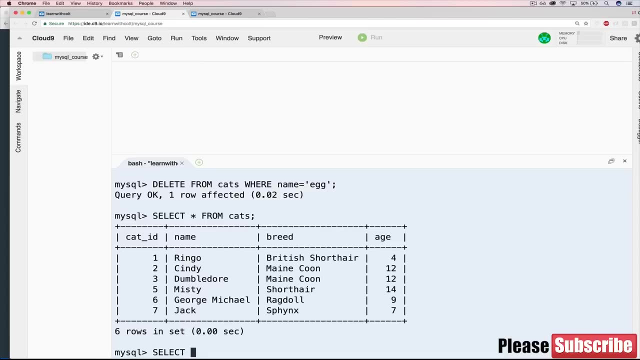 All right, give it a shot. So let's talk about solutions to these. The first one: to delete all four-year-old cats. all we need to do is start off, and you don't have to do this, but I like to start off. 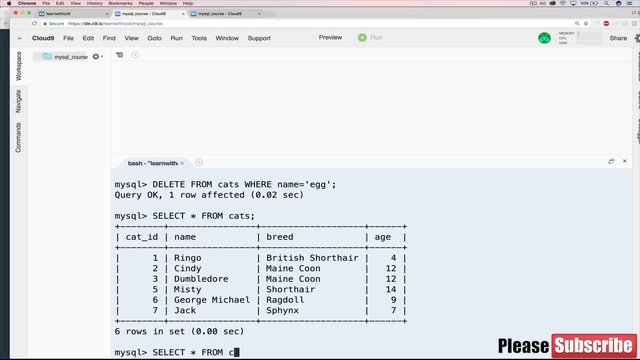 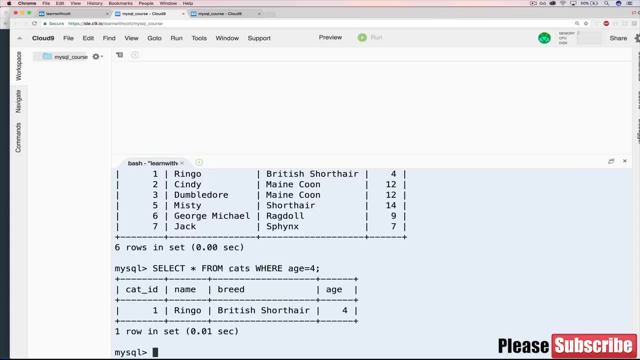 by making sure we're selecting things correctly. So select star from cats where age equals four. We get Ringo. Then I just like to copy this and do a delete from cats, And of course I forgot to add a space. but delete from cats. 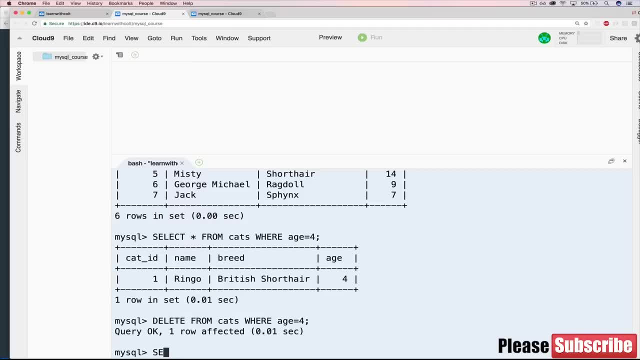 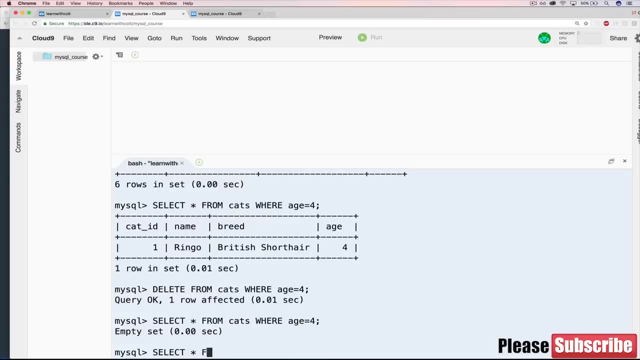 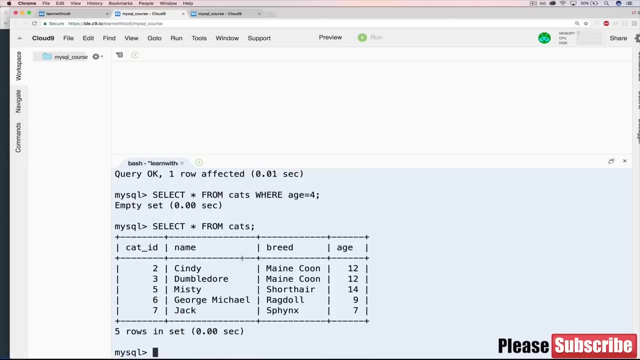 where age is four. Now, if we do a well, let's do our first select, We should see nothing. And if we do a select star, we should see that we're now missing number one, who was Ringo? by Ringo. 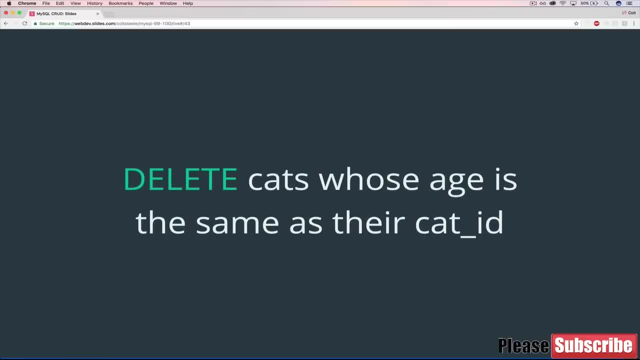 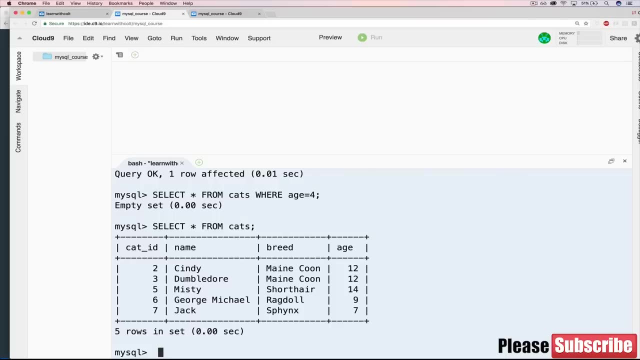 Okay, next up, delete cats whose age is the same as their cats with cat ID. So this one involved something slightly different, like I mentioned, where we're not just checking for a specific piece of data like breed equals Maine Coon or age equals 12,. 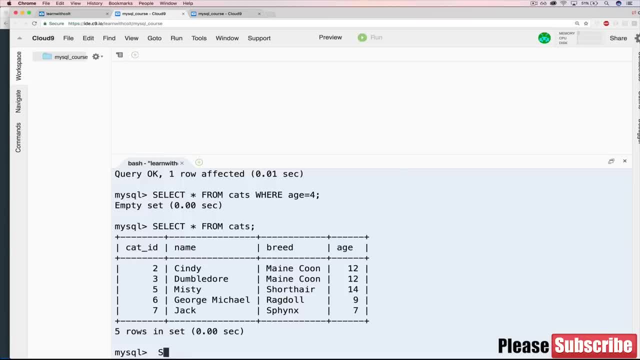 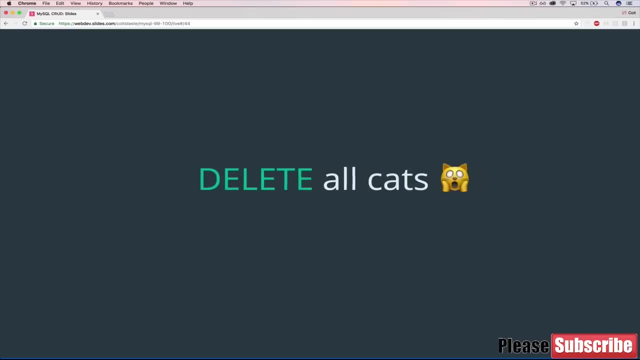 but we're checking where cat ID equals age. So we'll do a select. first select star from cats where cat ID equals age. or you could do age equals cat ID And we get Jack. cat ID is seven, age is seven. 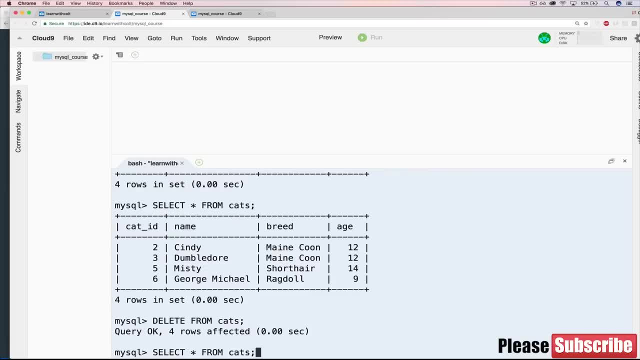 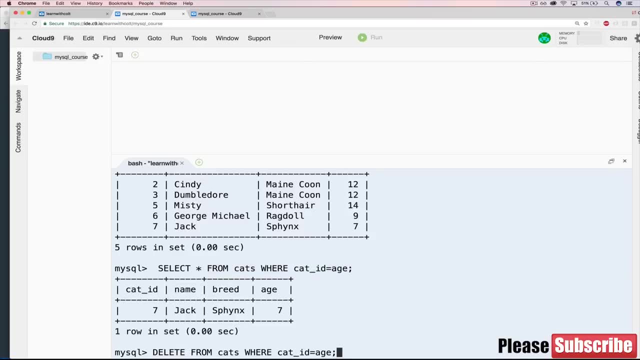 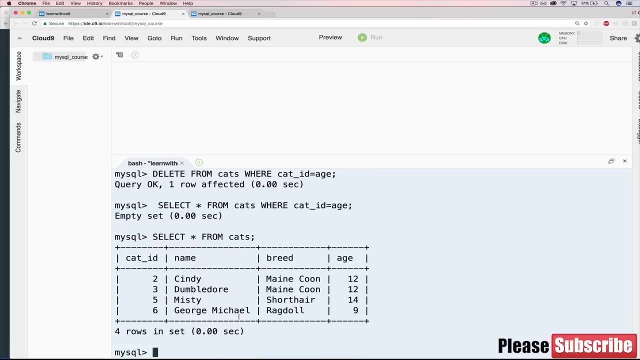 Great. So then we'll just copy this and do our delete from cats. where cat ID equals age, It says one row affected. If we try and select it again it's gone, And if we do a select star now, we're also missing Jack. 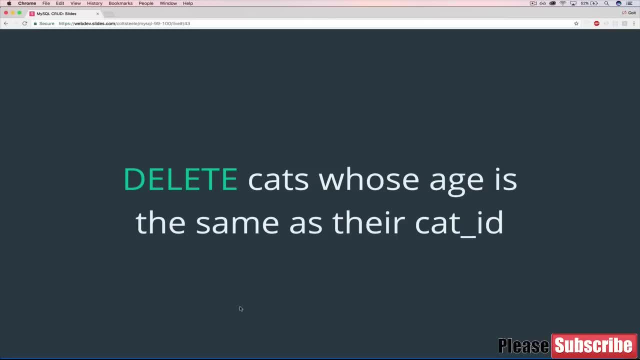 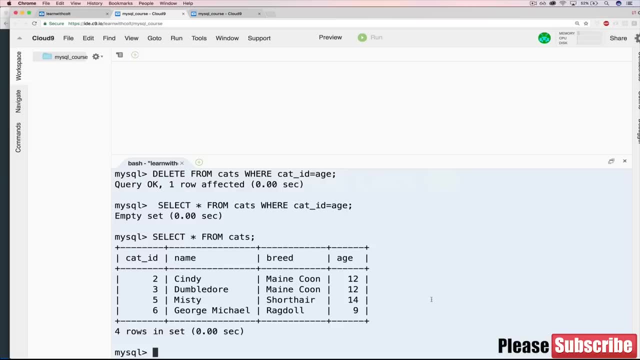 You can see we just have two, three, five and six, which leads us to our final example: Delete all cats. So this one is pretty straightforward. If we tried to do the equivalent select, it would just be select star from cats with no ensuing where clause. 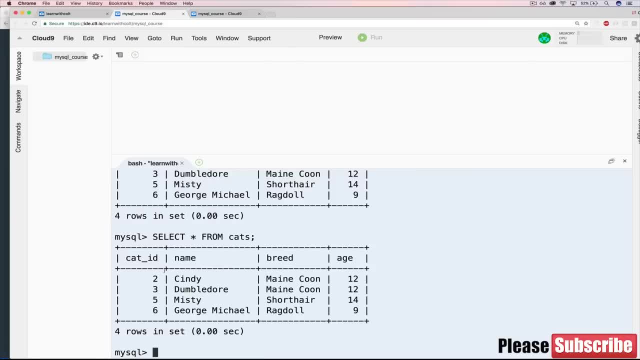 just like that. So to delete all of those? well, it's just delete from cats. All of our cats are being released at once into a land of rainbows and joy. We hit enter here. They're definitely 100% not dying. 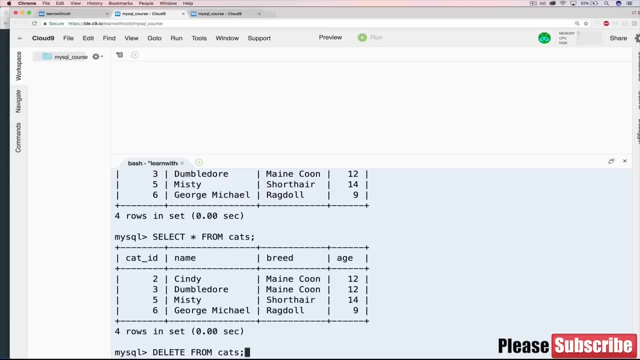 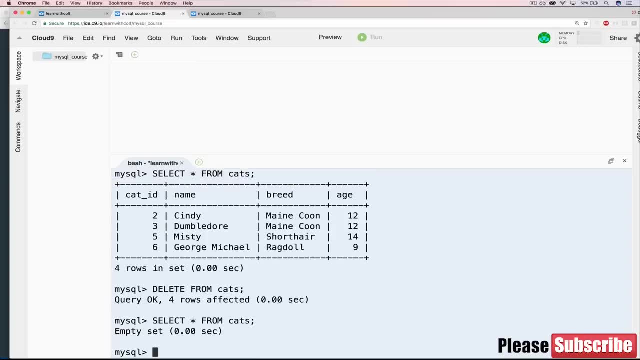 Nothing bad will ever happen here. Nothing bad will ever happen to them. Here we go, Four rows affected, Select star from cats, the moment of truth, And they're all gone and not dead. Okay, So we've now covered the C and the R. 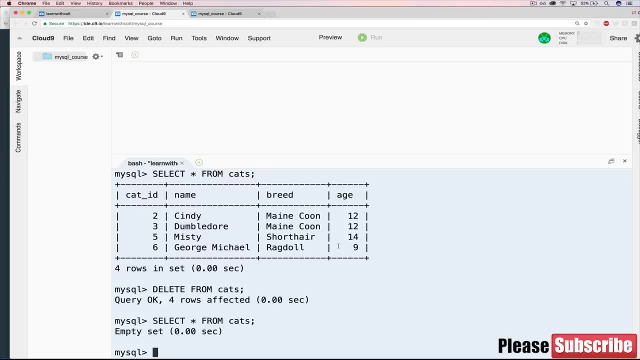 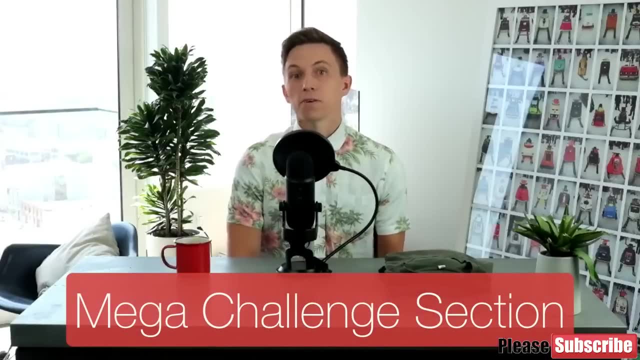 and the U and the D in crud. That spells crud, which means that we're done with this. Next up, we'll get some practice putting it all together. Hey, welcome to the next section. So this section is a bit different than everything else. 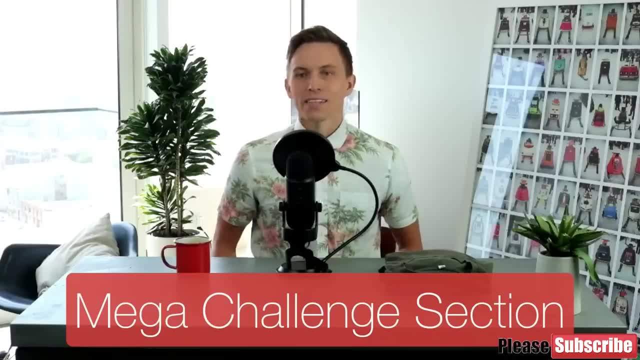 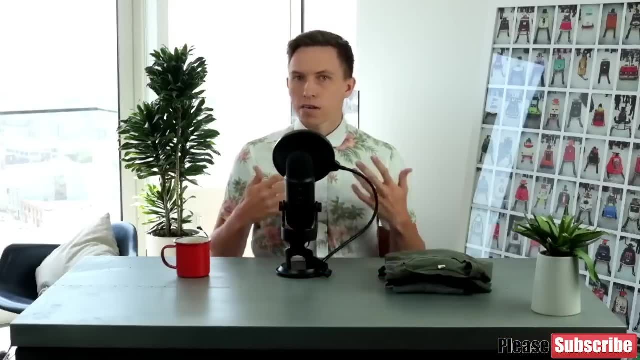 I mean, I guess you could say that every section, hopefully, but the structure is pretty different because it's all challenges, It's all exercises. So the way that this will work is you're going to practice all the commands you've seen up until this point. 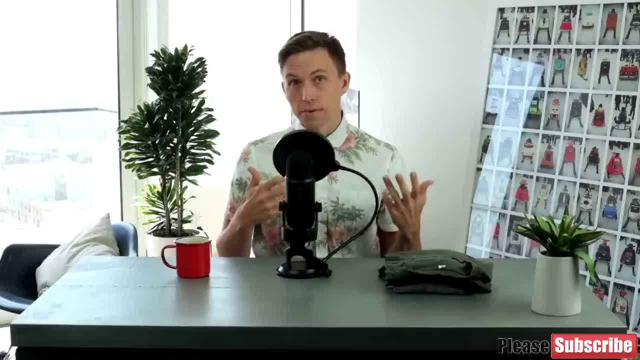 Everything from creating a database and switching and using the database to creating your tables and defining a schema, to then doing the basic crud operations we've talked about creating, reading, updating and deleting data. All that stuff, all those commands that are associated with that. 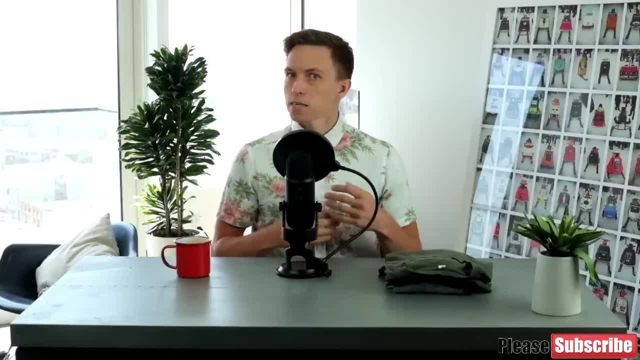 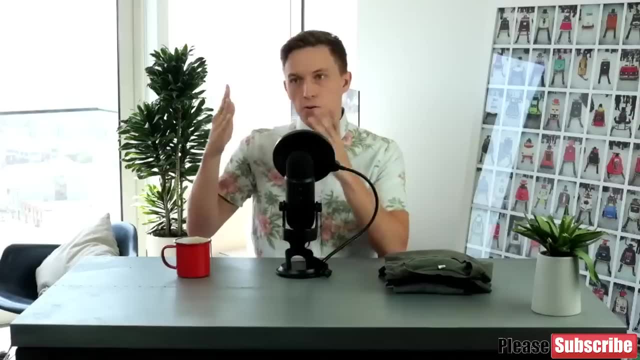 you'll be practicing them all at once in this section, And it's not just one giant video. I broke it up into kind of logical- hopefully, sections that make sense. You'll go through, you know, the create section. We'll create data together. 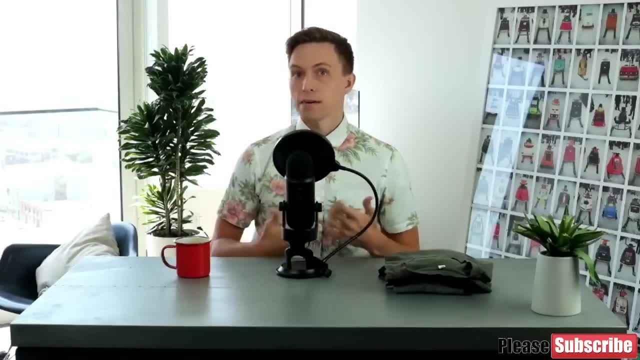 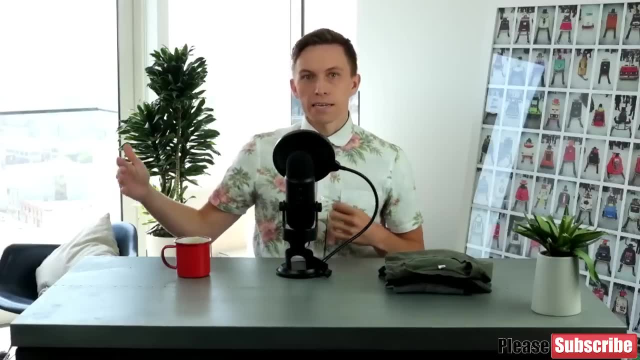 and then you'll do exercises with it And we'll be working with all the same data, so we get all the same answers, which is really important that you know, if you're following along and you're trying to update something, that your update looks the same as mine. 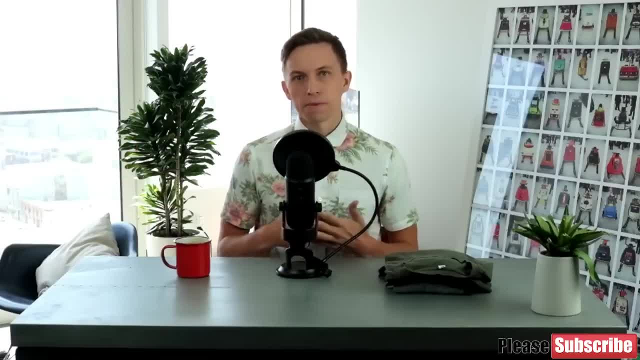 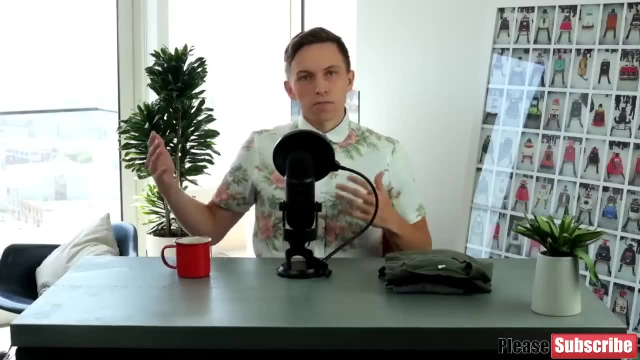 So the data that we'll be working with has to do with inventory management, has to do with, let's say, a clothing company, an online clothing retailer, or maybe just our closet. We're just doing an inventory of my closet. I need to figure out what fits. 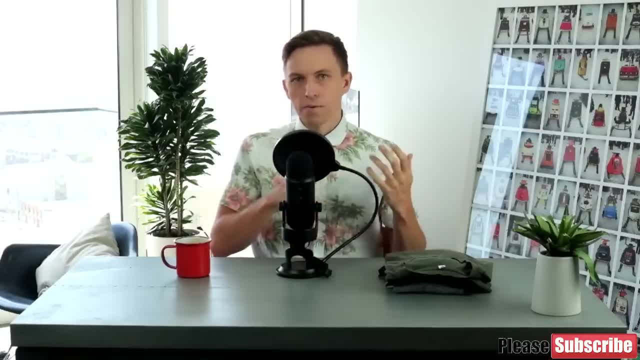 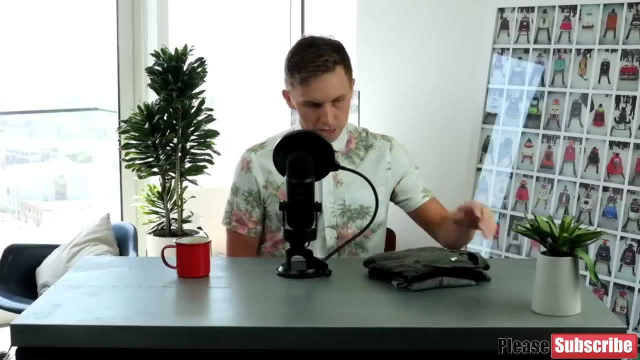 what doesn't fit, what colors are there? what shirts have holes? I don't know what to give away to charity, what to burn in a pile. if that's what you do, All that stuff, And you know we'll have different types of shirts. 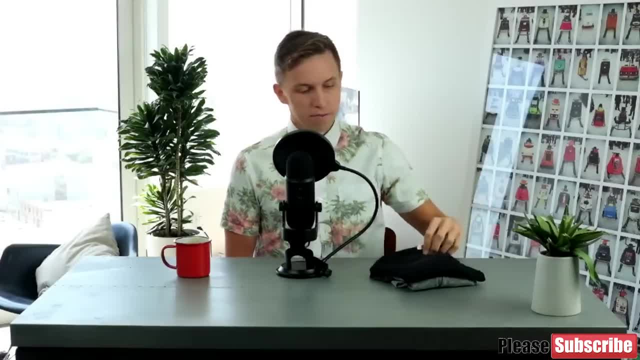 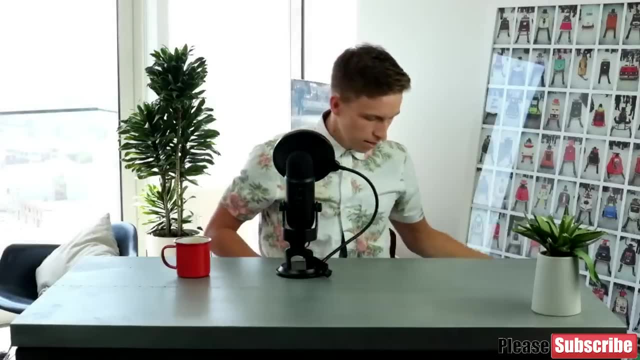 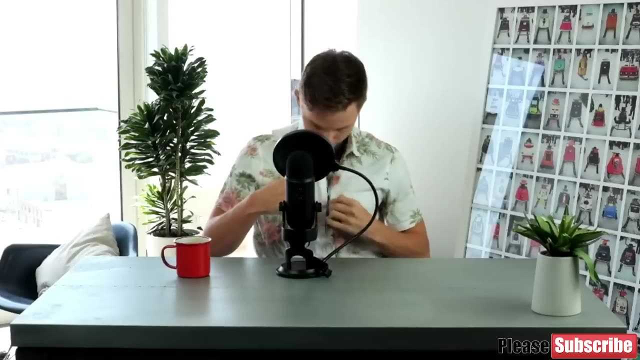 I got props again. You know short sleeves, We've got long sleeves and the underappreciated and elusive three-quarter length sleeve, Not to mention things like, you know, Hawaiian shirts, or even Hawaiian shirts of different colors too. I bet you didn't see that coming. 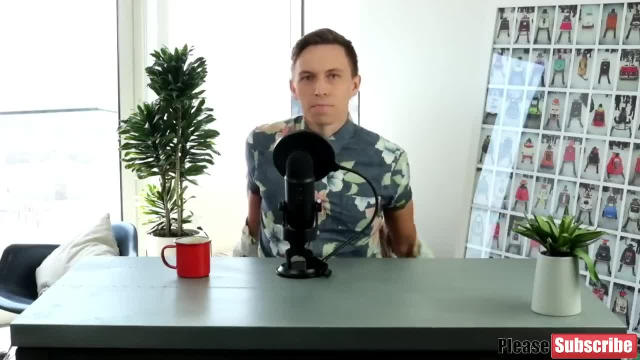 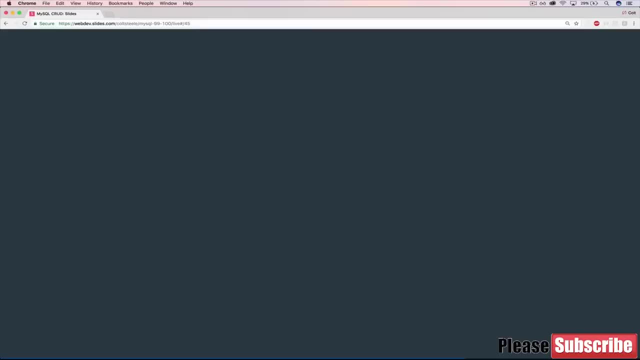 Look at that- another Hawaiian shirt. Yeah, I should probably stop this video, huh. So let's get on with the exercises Coming up. a whole bunch of exercises around shirts. All right, So we've seen the basic components of CRUD. 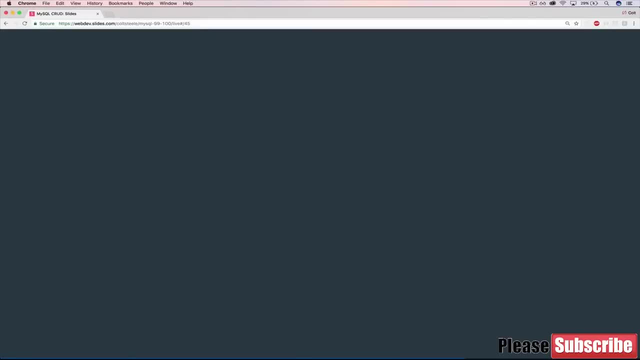 creating, reading, updating and deleting. You've learned how to do all those operations in SQL, And now it's time for the super, ultra, hyper, mega CRUD exercise. Actually, let me try that one more time. It's time for the super. 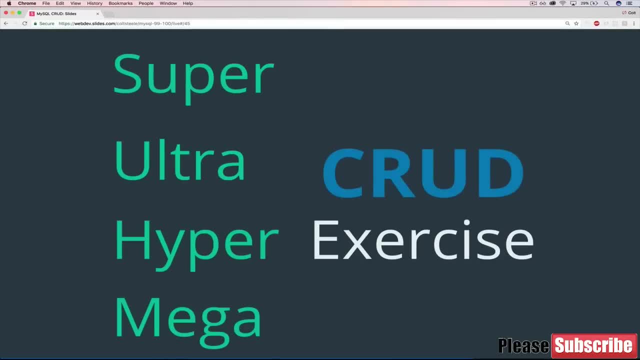 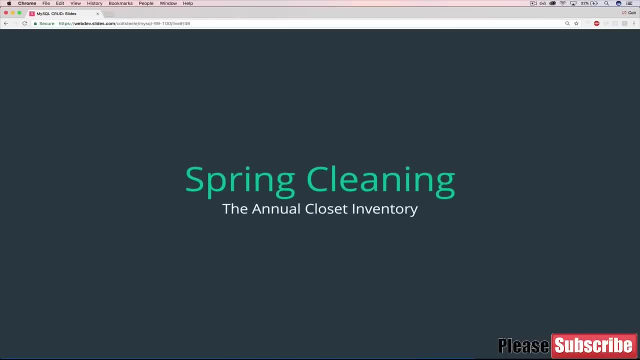 super, ultra, hyper, mega, mega, mega CRUD exercise. It's only been half a second, but I already regret that, So let's move on. So the idea here is that you're going to get to put all the different things you've learned to use. 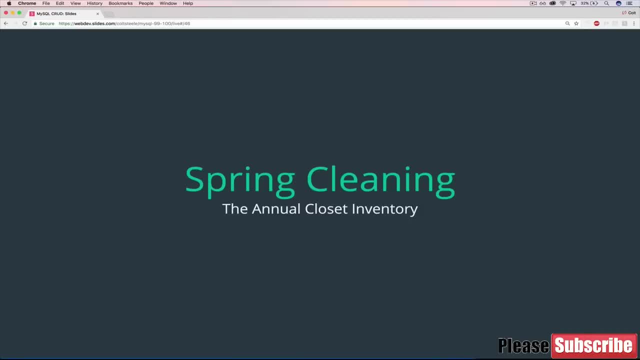 So this will be one exercise. In this case we're working on closet inventory- Super exciting, I know. So basically the idea is that if I or you or somebody has a bunch of clothing in their closet that they want to go through an inventory, 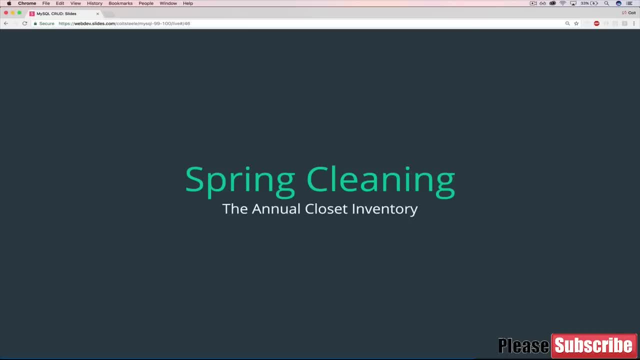 and figure out sizes and colors, And we're just focusing on shirts. so different types of shirts- tank tops, polo shirts, t-shirts and so on, And we can go through and we'll just perform some basic operations on them. I do want to add a note that 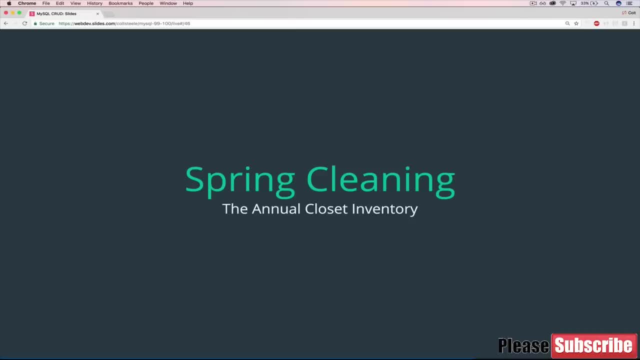 I know that up until now our data has been sort of trivial, And this included t-shirts- is not that exciting or that realistic. really, We still don't have the pieces to go into complex real-world data that you would see in a web app. 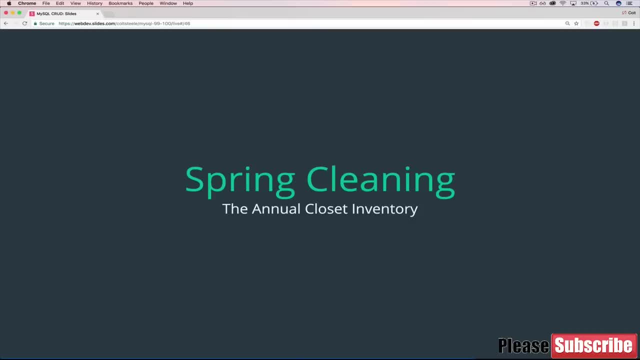 But we will get there And so hold tight. I promise we'll be seeing a lot of real-world, potentially more exciting, definitely more challenging data. So we're working with Spring Cleaning and you're going to have a bunch of operations to do. 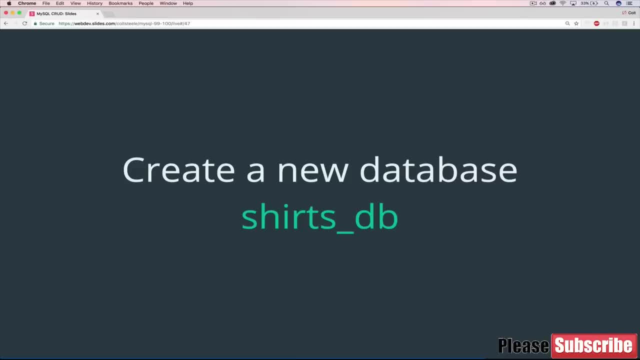 And the first one is to create a brand new database. So think back to how we did that. No more working in the CATS database. We need a new one called ShirtsDB. So create that, And then the next step is to create a new table called Shirts. 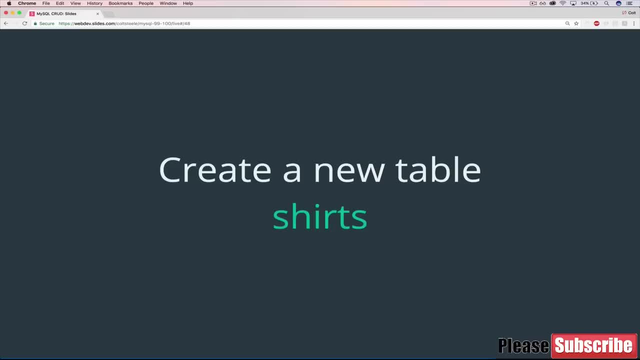 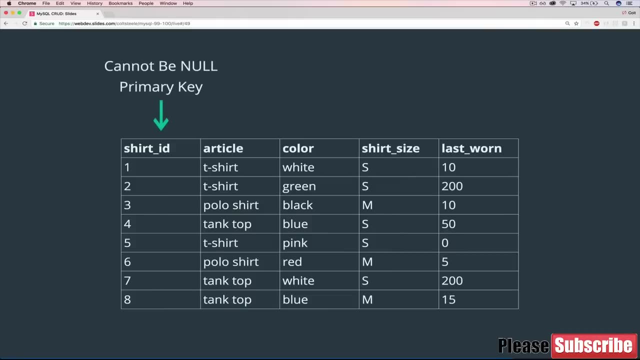 And to do that you need a little more information. You need to know what does that table look like. So here you go. Here's a graphic representation. We've got a shirt ID, which cannot be null and is a primary key. 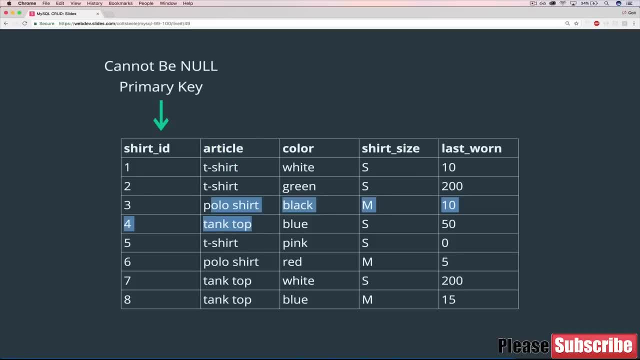 We have article, which should be something like t-shirt or polo shirt or tank top: It's text. Then we have the color of the shirt, which is also text: White, green, black, blue and so on. We have the shirt size. 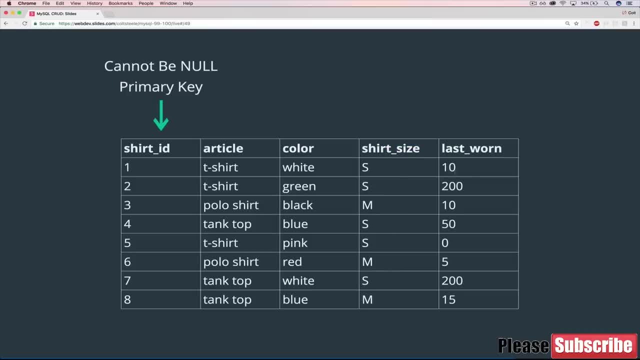 In this case, smalls and mediums Text. And then we have last. Oh, actually, before I move on, I do want to call your attention to the fact that I did shirt underscore size rather than just size, And that's because size is. 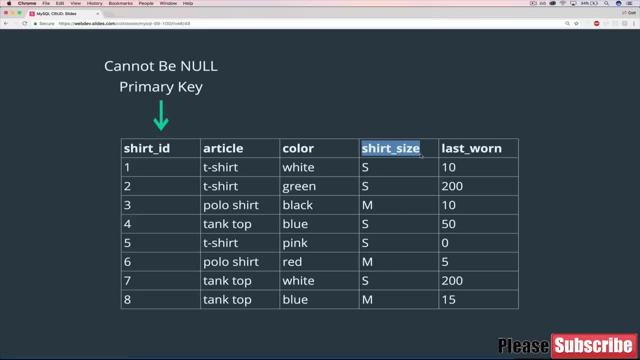 a bit of a reserved word, So you can still use it, but it's a word that MySQL uses internally- Size- And so it's better to avoid any conflicts there. So I just went with shirt size, And then last worn is a number. 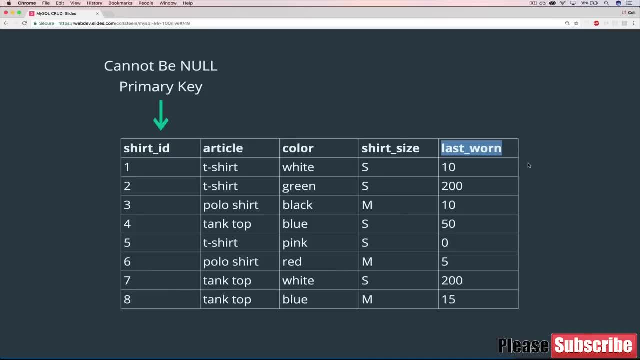 And that refers to roughly how many days ago the shirt was last worn. So the idea is that we would inventory our closet. Maybe you do this, Maybe you don't, But you go through and you figure out what you don't wear all that often. 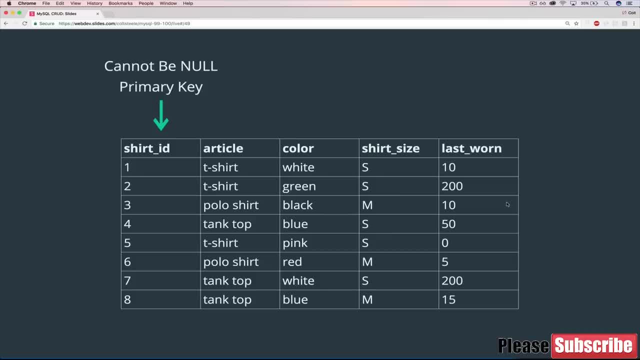 And then either sell it or donate it or, I don't know, make tie dye with it, Whatever you do. So that's what we're trying to calculate, or what we're trying to store here, And it's just a number for now. 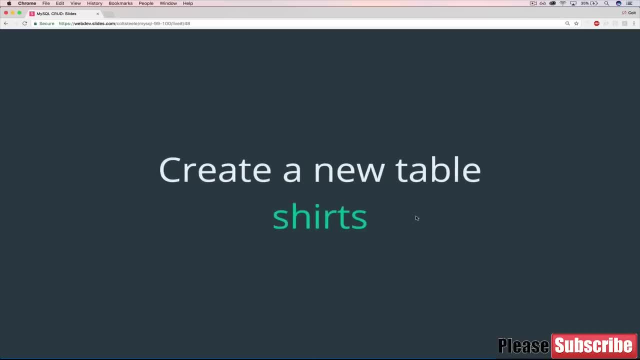 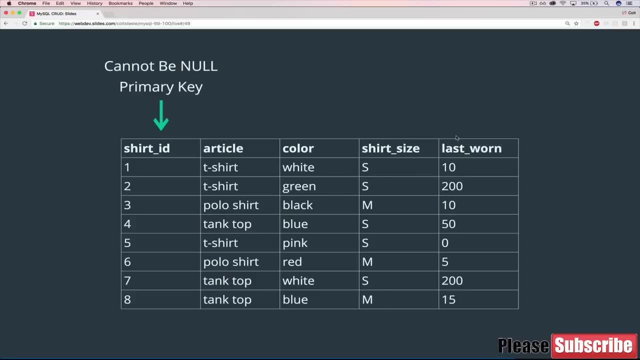 So create that table- It should be called shirts- And once you do that, you can move on to the next step, which is getting the starter data in there. So I want all this data in the table, but I don't want you to have to type it up yourself. 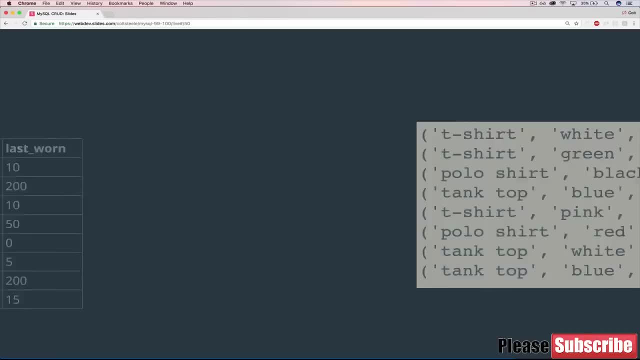 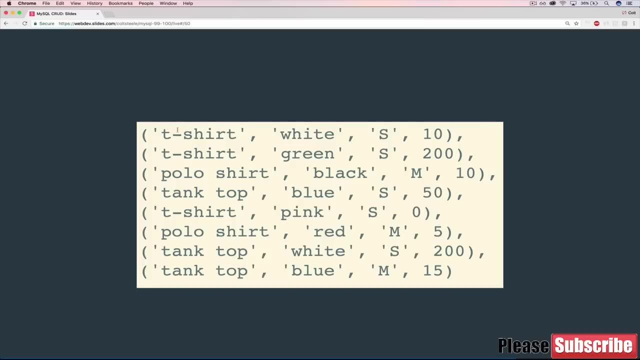 It can be obnoxious to insert that manually, So I've given you basically a starter seed data that contains the exact same thing. So a white T-shirt that's small with 10 days ago, So you can see it's the same as this first shirt here. 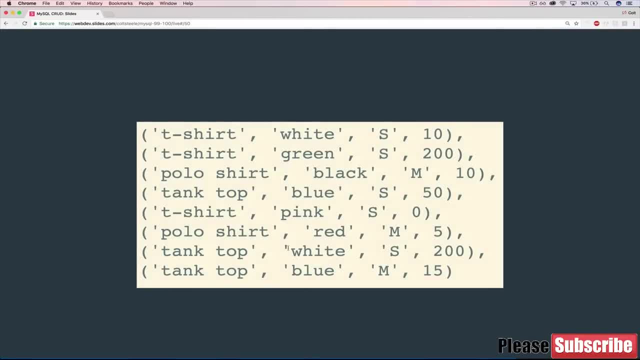 And I've done it for all eight, So you could copy this- It's in the text of this video as well- And then what you could do is just insert it all at once. So remember how to do a multi-insert. Get all that data in there with a single line. 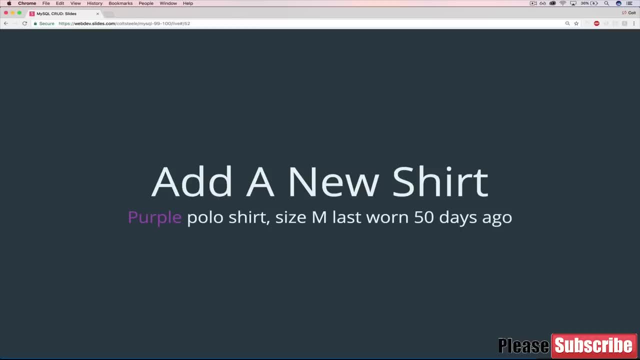 And then the next step is to add a single new shirt. So insert something manually, not using a multi-insert, but just one at a time. A purple polo shirt that's medium, that was last worn 50 days ago, All right, So then, once we have those nine shirts in there, 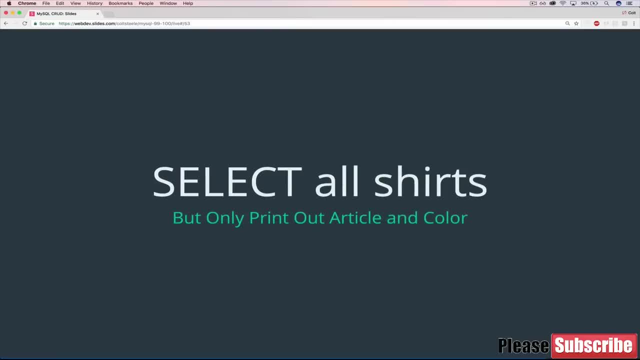 we can now start to do some stuff with them. First thing we'll do is select all shirts but only print out article and color. So we should only see T-shirt purple, polo shirt black. We don't want to see ID, We don't want to see size or last worn. 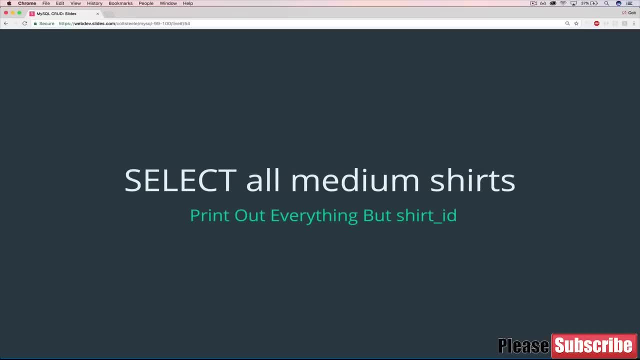 Then, once you do that, the next step is to select all medium shirts, So all shirts that have size of medium, and print out everything you want, Everything but the shirt ID. So we want all of this here: Article: color, shirt size last worn. 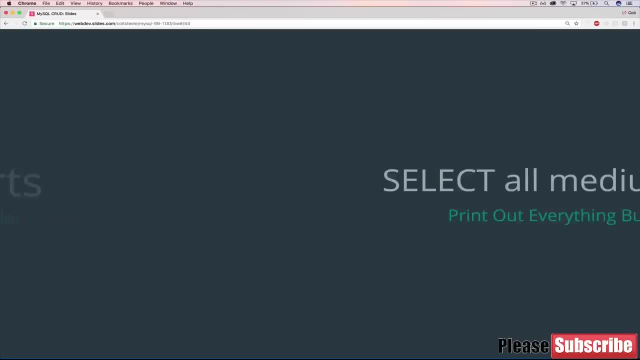 but not this, But only for the mediums. Okay, Then next up, we're moving on to update. So we've done the create and the read. We're working on update now, which is update all polo shirts to be size large. 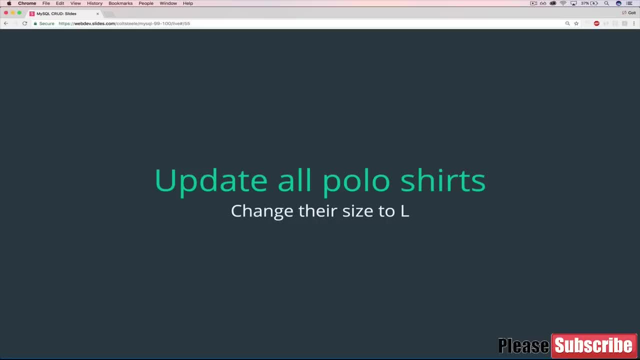 Maybe- I don't know- you realize that the company that makes your polo shirts, it might say medium on them, but in reality they're pretty large And so you want to update your database. It's a dumb story, Let's just go with it. 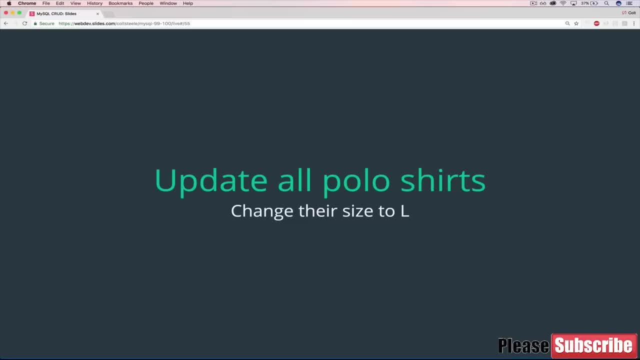 So change their size to large. So that's where article equals polo shirt. Next up, update the shirt that was last worn 15 days ago and change last worn to zero. So this would mean there's a shirt that was worn 15 days ago. 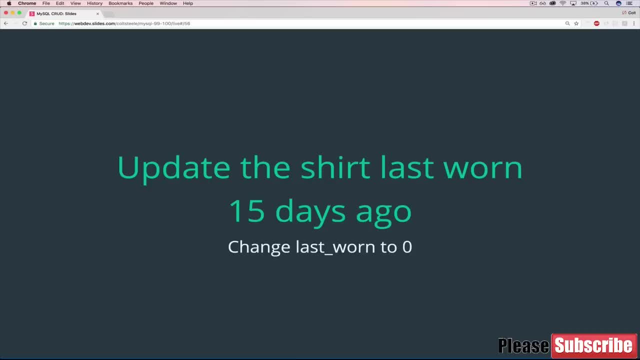 that we decided to wear today. So we're going to change the database to say last worn is now zero. So once you do that, now our final update. we had a bit of a mishap. We were doing laundry. We took all the white shirts. 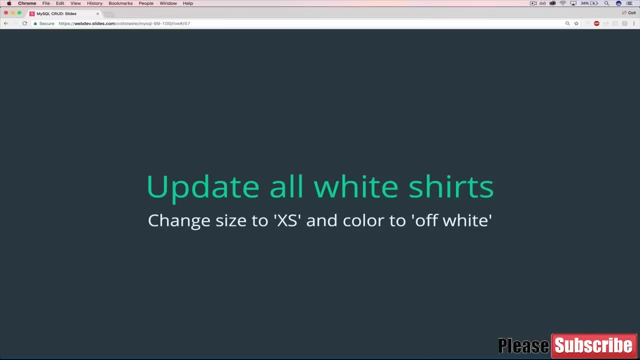 and we washed them with, I don't know, some colored stuff that we shouldn't have, And we shrank them at the same time. So we have a double update here. You need to update all the white shirts to now be an extra small size. 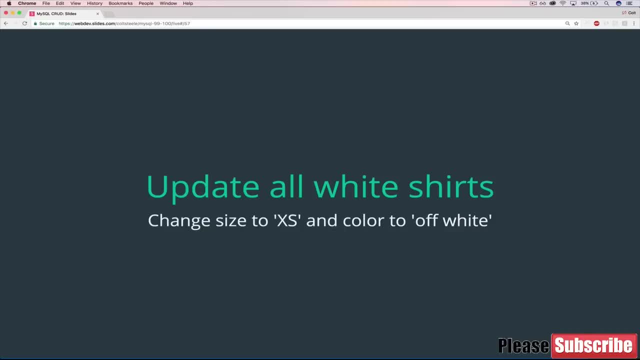 and their color is no longer white, but it should be off white, So you need to update that. So you need to update both of those at once with one line, just to be clear. All right, Next we're deleting, So delete all old shirts. 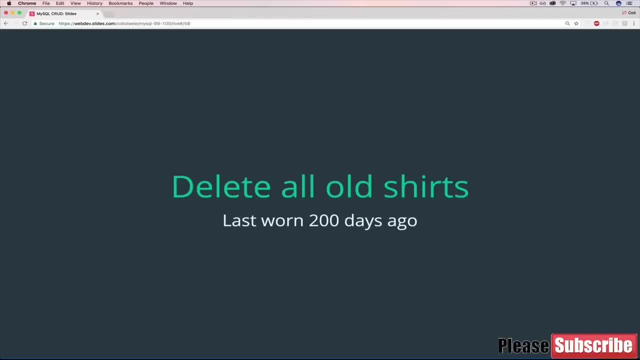 And in our case, old just means if it was worn 200 days ago or last worn 200 days ago. We will see very shortly how you can do things like delete all old shirts that have been last worn greater than 50 days ago. 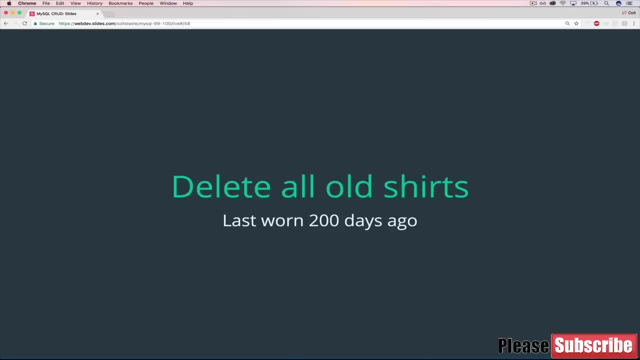 But for now we're doing exactly 200 days. Okay, Next up. our taste has changed. We've decided we no longer like wearing tank tops. We don't like the person that it turns us into, So we're going to delete all tank tops from our database. 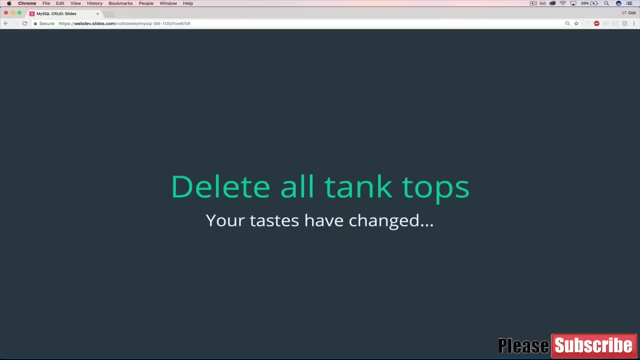 So delete all shirts where article is tank top. Then, finally, catastrophe strikes. We have to delete all shirts. I'll let you decide why, but we need to delete all the shirts. That doesn't mean delete the table or the database, Just delete the shirts in the table. 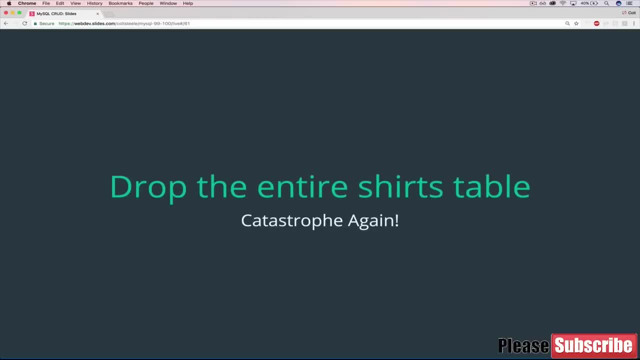 So it should be an empty table. Then, finally, drop the entire shirts table- Another catastrophe, So it should be an empty table. at this point, Drop it entirely And that's it. So go through all those steps. I recommend just pausing the video as you go. 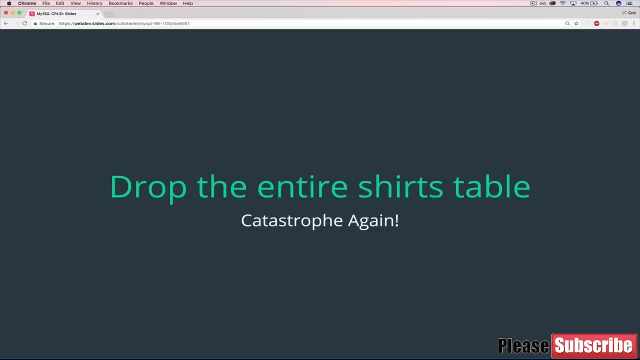 Make sure you do them, And then, if you'd like watch the solution to see how to do it or how I did it, Okay, All righty, Let's go through the solution. Spring cleaning: We're cleaning our closet inventory. 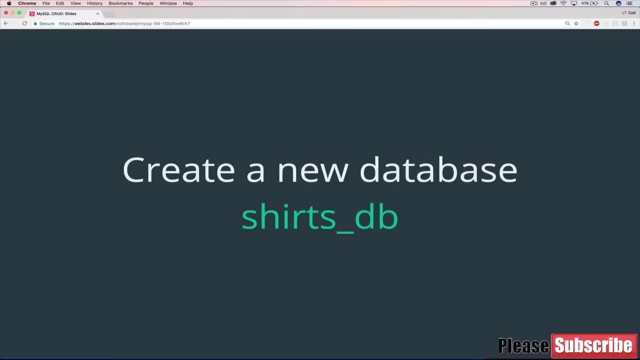 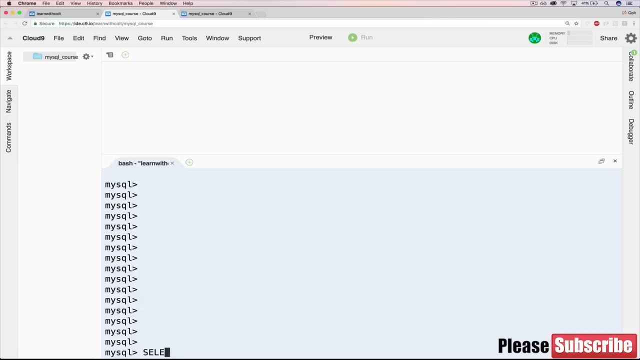 And the first step was to create a brand new database called shirts DB. So if we hop over to cloud nine, if we just check what database we're using, remember we can do select database. We're using cat app, So we're going to make a new database. 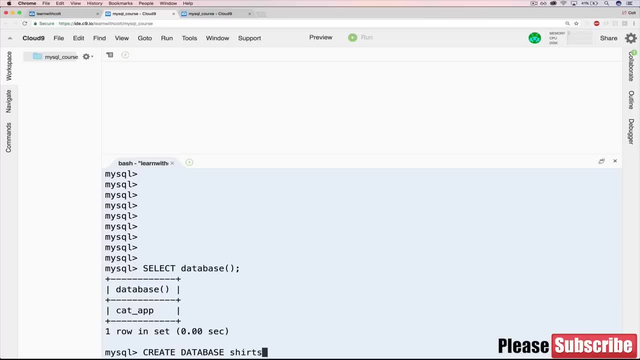 Create database And we wanted to call it shirts underscore DB semicolon. Now, if we do show databases, you can see we have shirts DB down at the bottom. All right, So the next step: we need to use shirts DB, just like that. 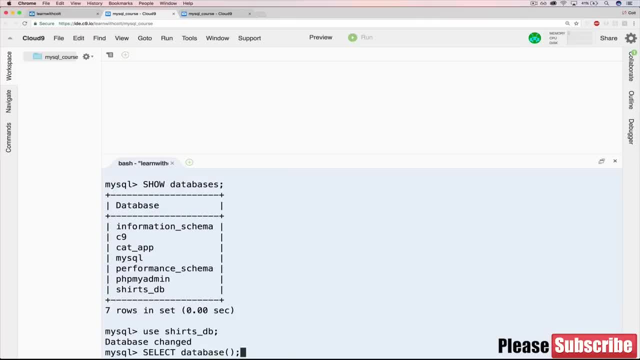 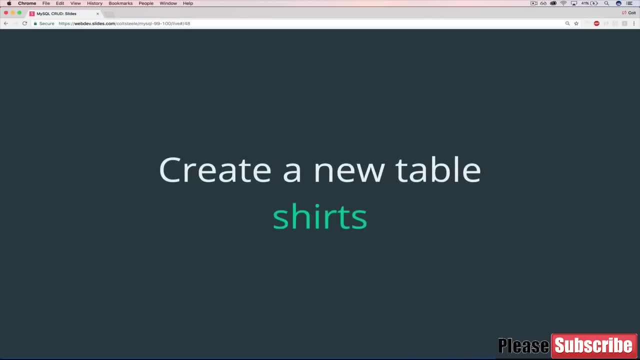 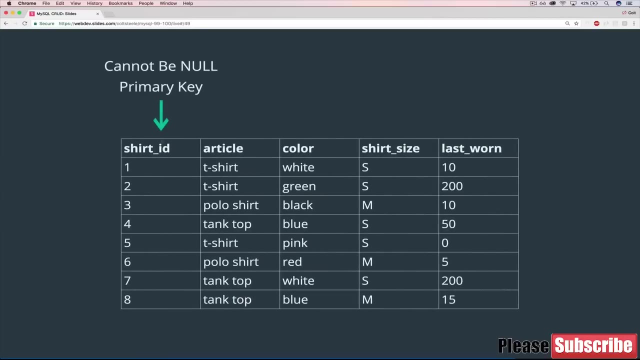 And now, if we run that same select database line, we're currently using shirts DB. Okay, So now this is probably the longest thing you'll have to type. We need to create a new table, We'll call it shirts And it needs to have these five columns. 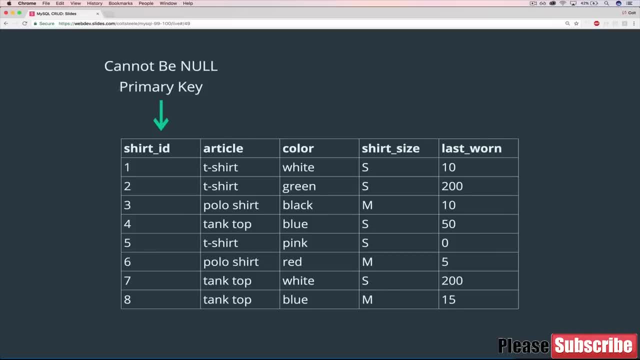 Shirt ID, which cannot be null and is a primary key, which means that we'll have it auto increment as well. Article which should be varchar. And let's just for simplicity say: all of these have 100 character limit Color. 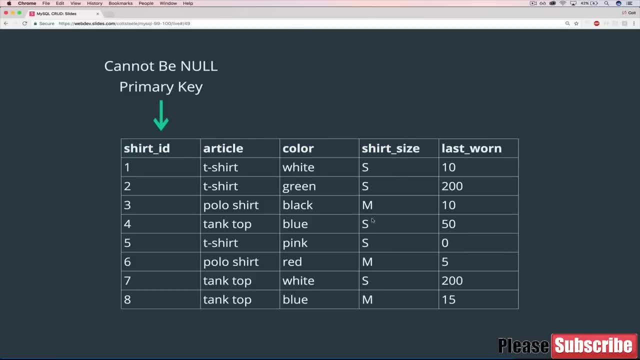 varchar 100.. Shirt size: Yes, we could have kept it short, but maybe you might have a shirt size that's small. spelled out the full word rather than just the letter S, So we're not going to limit that either, for now. 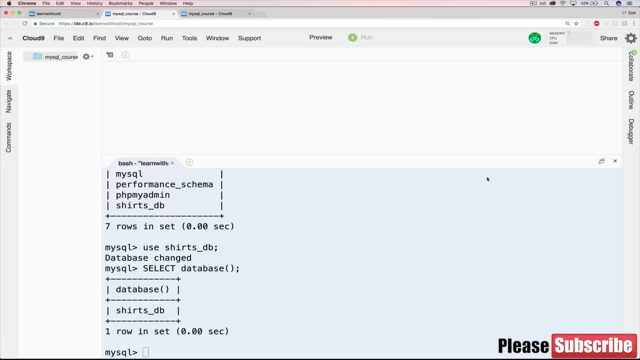 Okay, And then last worn is an int, So let's try it. We'll do a create table shirts And I'm going to do this on new line here, And the first thing that we have. let's start with shirt ID. 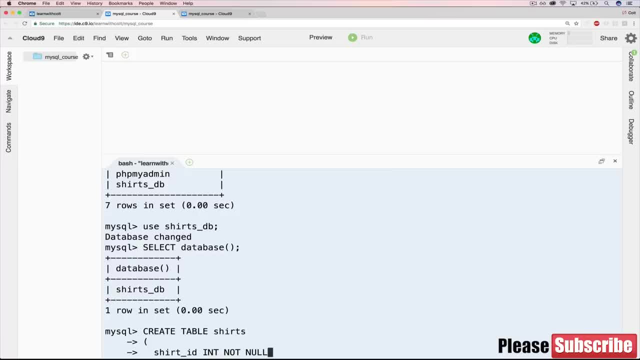 which should be an integer, not null auto increment. Next we're going to move on to article, which is a varchar 100.. And then after that we have color, which is also varchar 100.. Then we have shirt size. 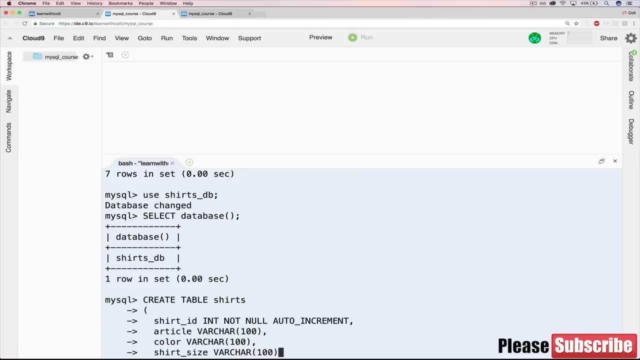 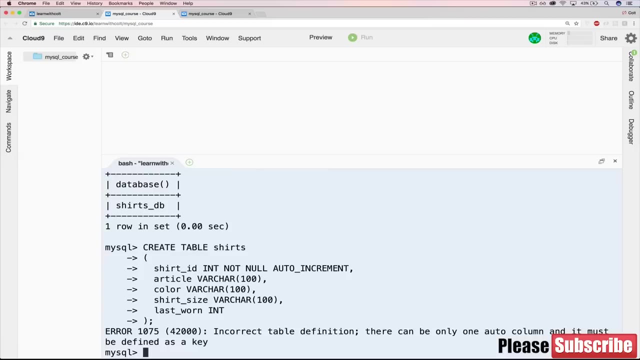 which is also varchar 100.. And finally, we have last worn, which is an int, Just like that, And we'll close our parentheses And then we'll add our semicolon. And I forgot something Which I did not do on purpose. 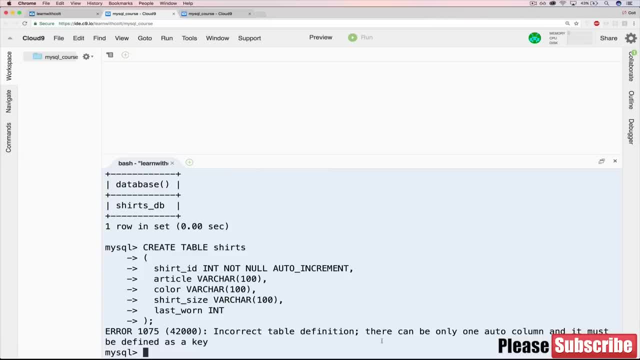 But if we look at the message, it says incorrect table definition. There can be only one auto column and it must be defined as a key, And so I'm missing the primary key definition at the end, which this is actually a helpful error. 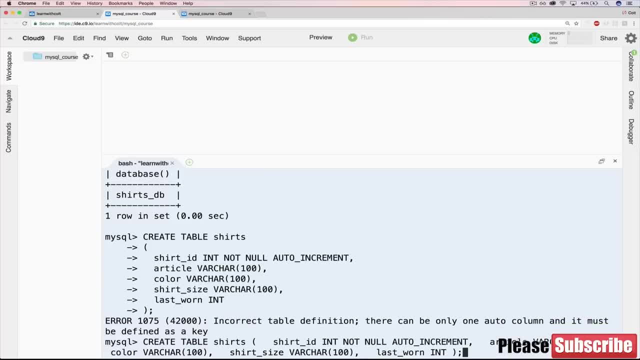 Oftentimes these error messages aren't that useful, but this one tells us exactly what we did wrong. So I'm going to recall that line And then at the end I'm going to add comma- primary key. And then our primary key is shirt ID. 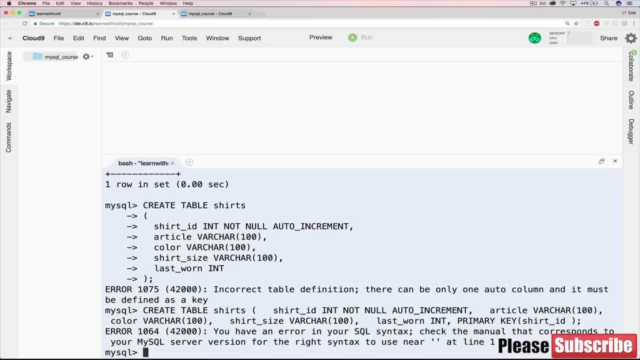 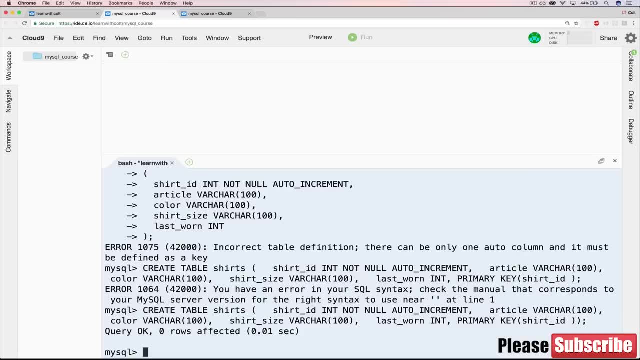 Just like that. Now, if I hit enter- and would you look at that- I left off the last parentheses again, So we have another error. Okay, so now if we hit enter here, it worked. If you'd like to see a nice cleaned up version, 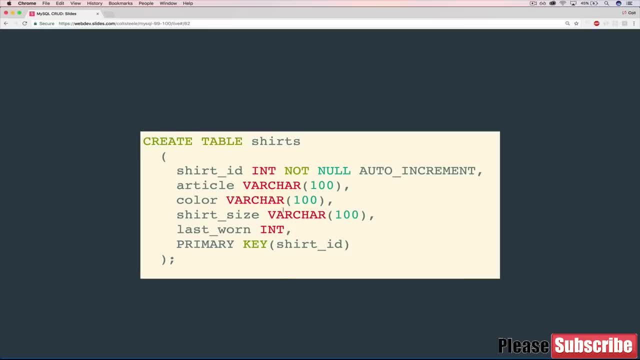 of what this actually looks like here. I have it here. So create table shirts. shirt ID. int not null. auto increment. article: varchar. color varchar. shirt size varchar. last worn int. primary key shirt ID And the semicolon and the correct parentheses. 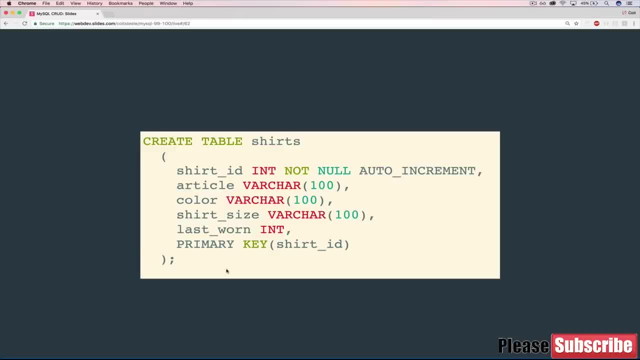 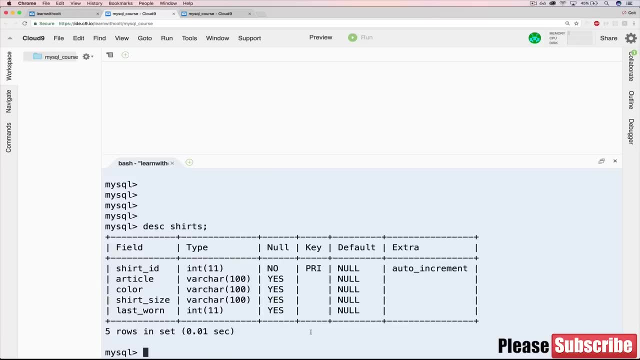 closing it out, And that should do it All. right, And if we wanted to double check that things worked, we can do our describe shirts And you can see we have what we expect. So the next thing is to get all of this data. 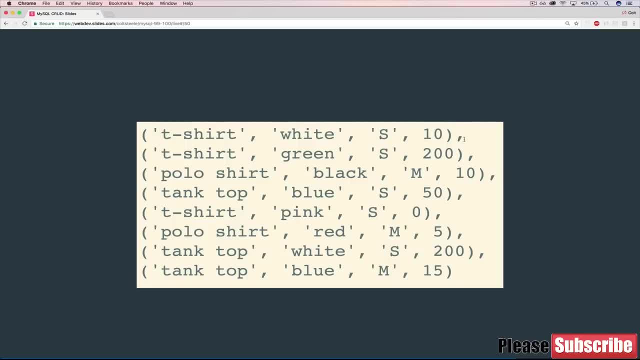 in our database. So I gave it to you as this comma separated list where things are all in the same format, where we have parentheses for one shirt and then inside of that we have article first and then color and then size and then last worn. 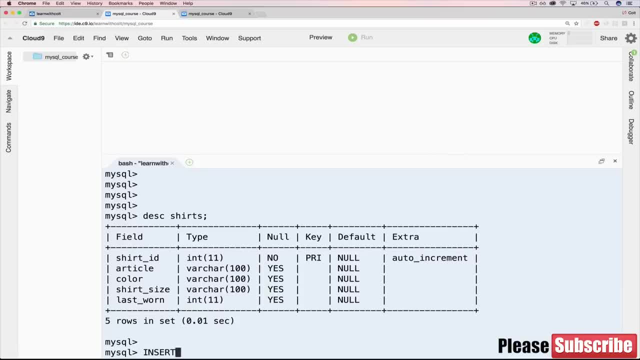 So we can insert using that format. So we'll do an insert into shirts And we have to specify: We're doing article first, Then we're doing color, Then we're doing shirt size And then finally we're doing last worn. 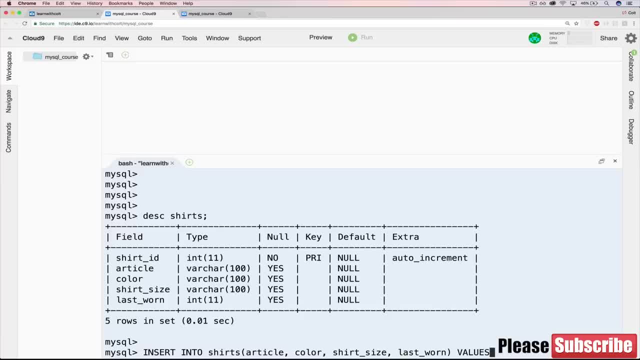 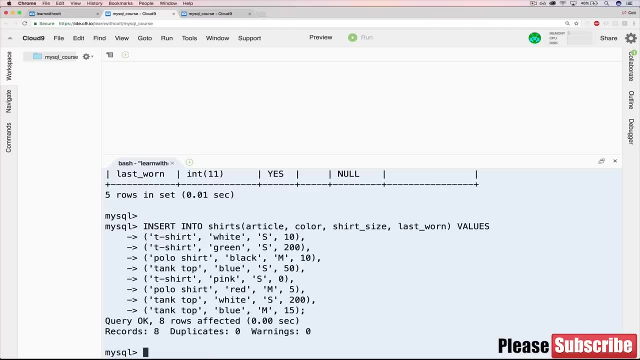 And then we need our values. And I'm just going to hit enter for now And I'm going to paste that giant list And we need a semicolon at the end And we hit enter- Good, No mistakes. this time It says records eight. 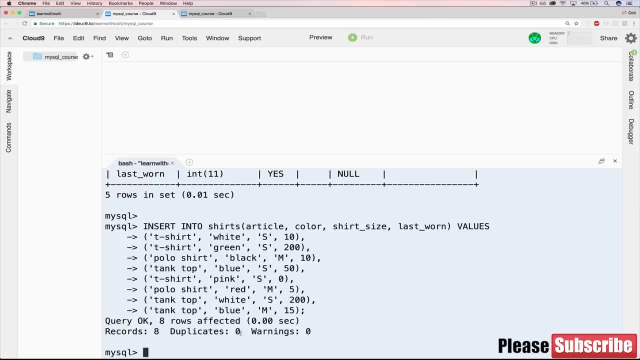 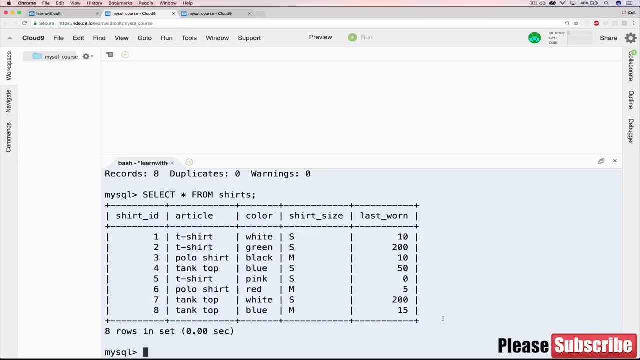 eight rows affected. Okay, So if we wanted just to double check, we can do our select star from shirts And we get the data in there that we should have, And then the last thing we need to do is to add a new shirt. 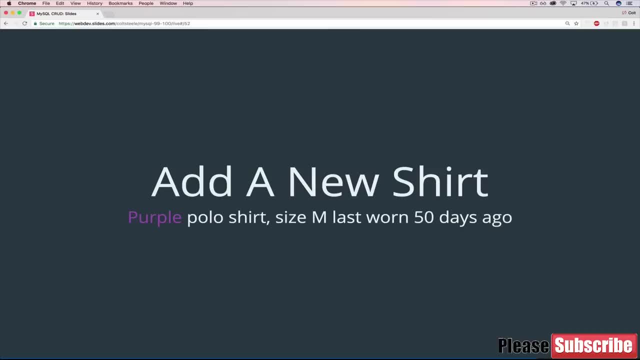 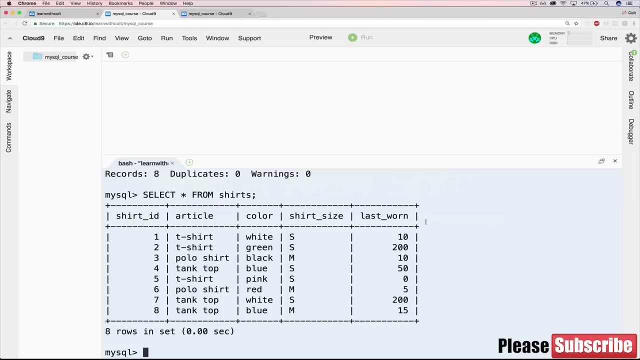 So manually one shirt rather than bulk inserting. It should be a purple polo shirt that's medium. that was last worn 50 days ago So I didn't specify what order you needed to insert into, So I don't really care, But we'll do insert into shirts. 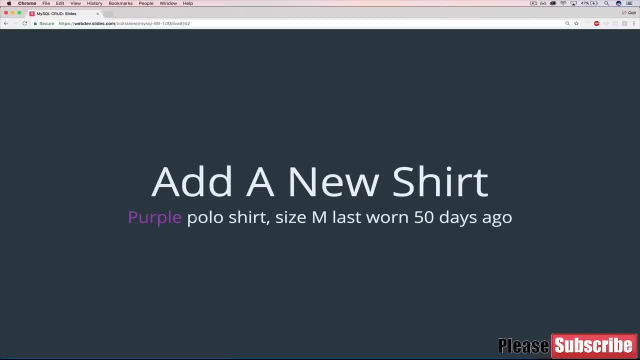 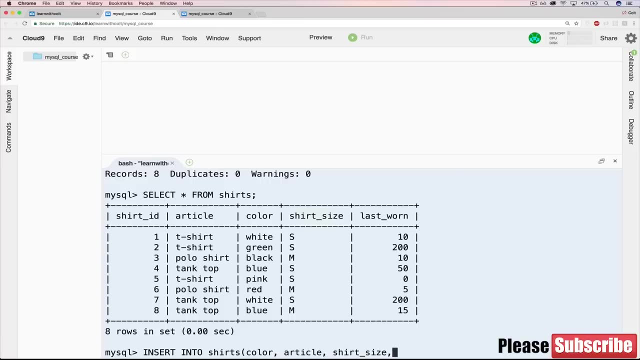 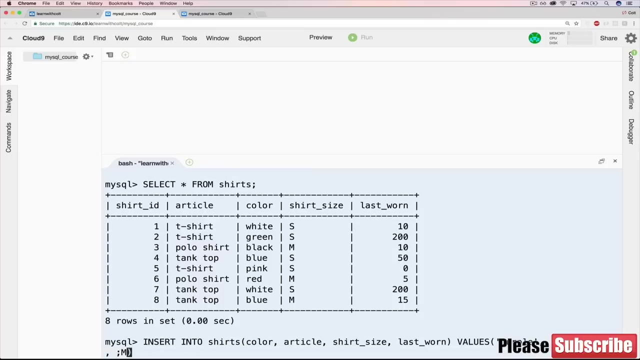 And we'll do color, because that's how I specified here: Color, then article, then size and then last worn. So color article shirt, size, last worn, Like that Values, And it's purple polo shirt, Comma medium. 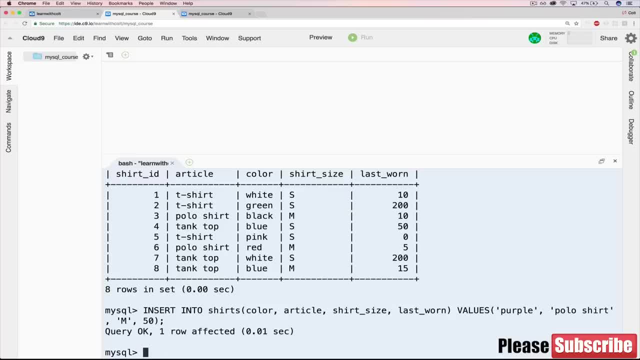 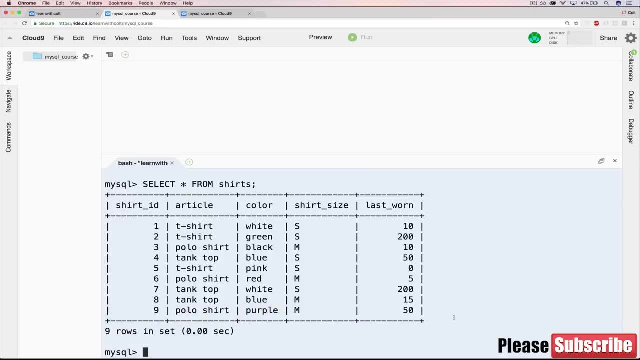 Comma 50.. Just like that, Okay, And if we do select star, we should see that new polo shirt down there. It's purple medium. 50 days ago we wore it All right, So we've now wrapped up the create part of CRUD. 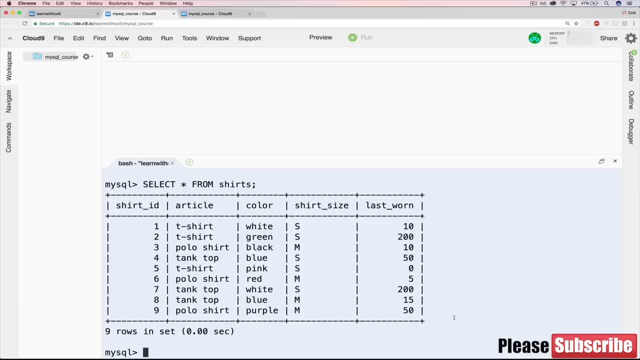 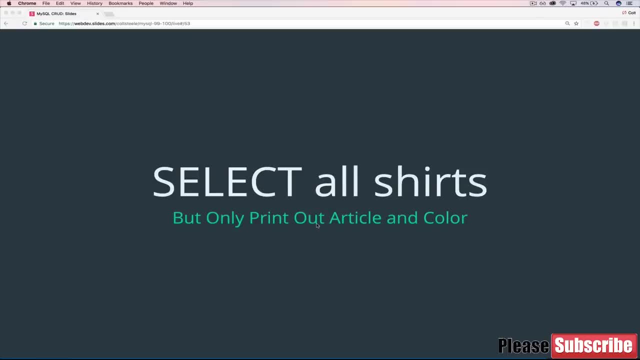 We saw how to create the database. We created a new table, We inserted data into the table. Now we're moving on to reading. So this is the read solution. Basically, it's a bunch of select statements we're going to write. 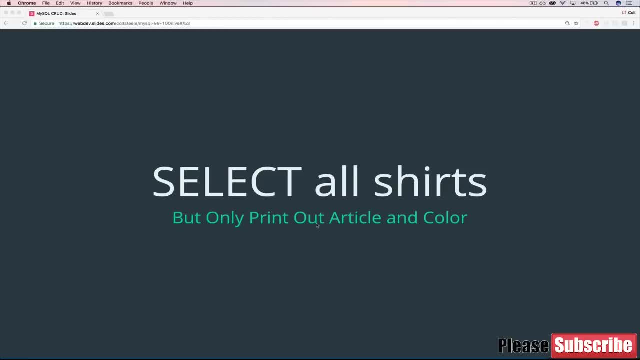 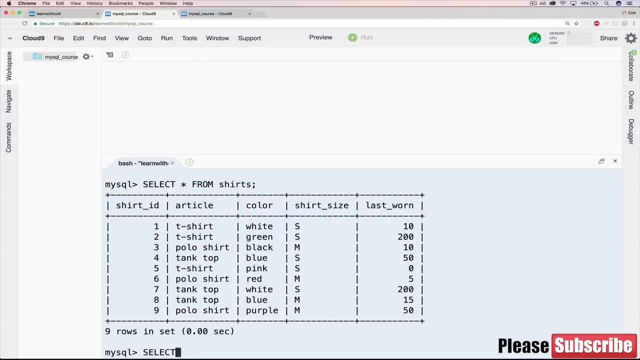 So the first one is to select all shirts but only print out their article and their color. So, back in Cloud9, all we need to do is select And rather than just select star, which gives us everything from all shirts. I mean, this is correct in that we want all shirts to be listed. 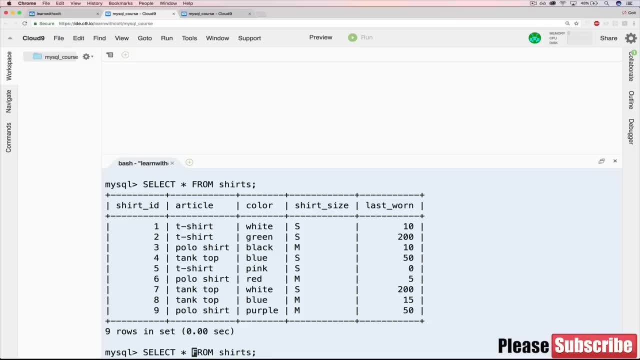 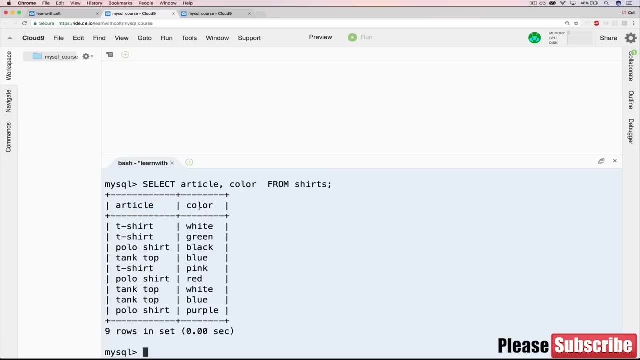 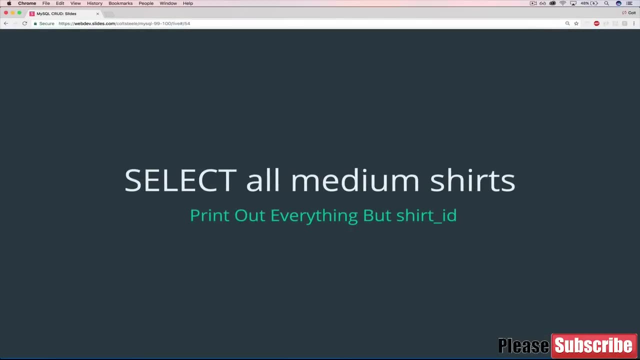 but we wanted to narrow down the fields. we get which was article comma color. And there we go. Article color: T-shirt white, Polo shirt black, Tank top white And so on. Next up, select all medium shirts. 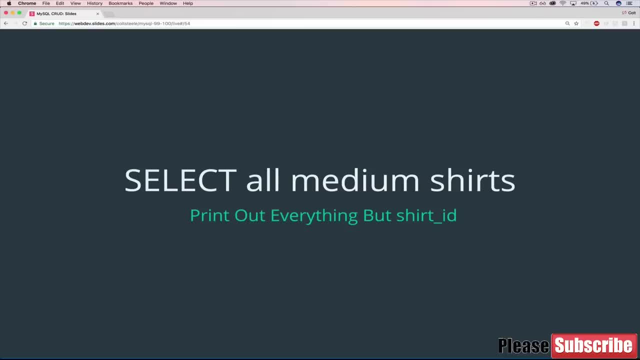 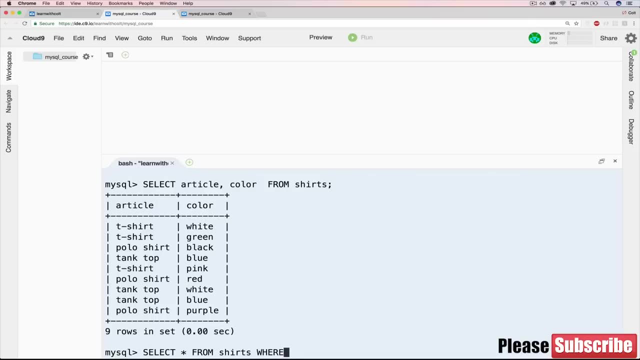 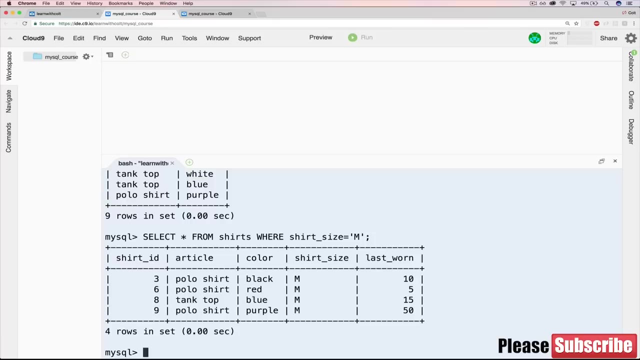 but only print out shirt ID. So that's all we want. So let's start off by just getting the medium shirts. So select star from shirts where. And then we need to do a shirt size equals medium, Just like that, And we'll hit enter. 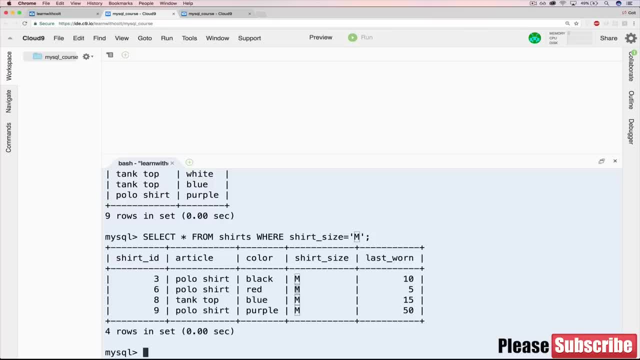 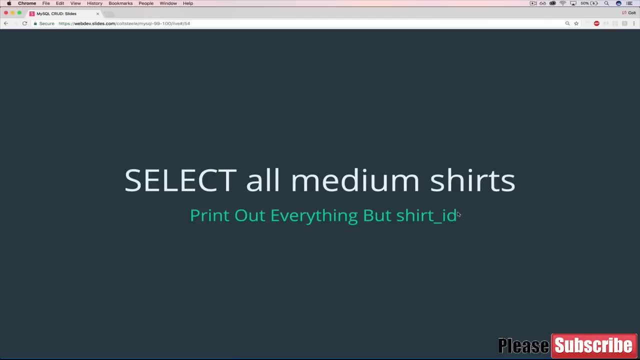 And we get four shirts that have shirt size of medium, But all that we want is everything excluding the shirt ID. Just a moment ago- I think I said it backwards- We want everything but the shirt ID, which means we need to list everything we want out. 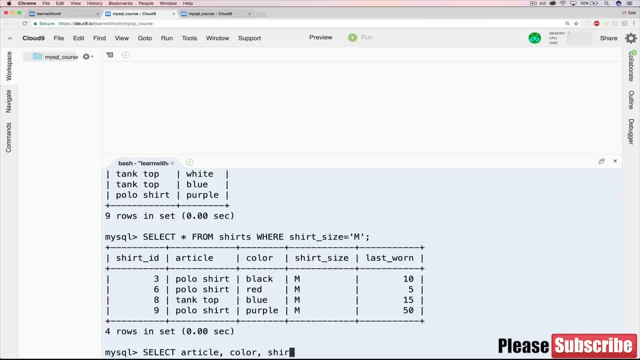 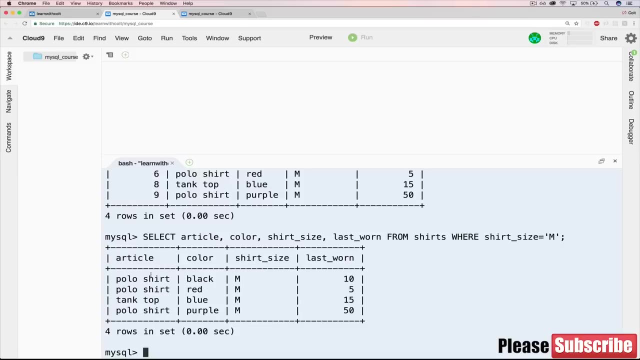 So select article: color, comma, shirt size, comma, last worn, And then we can just copy this from shirts where shirt size equals medium. And here we go, We have all mediums And we have the four columns we're looking for. 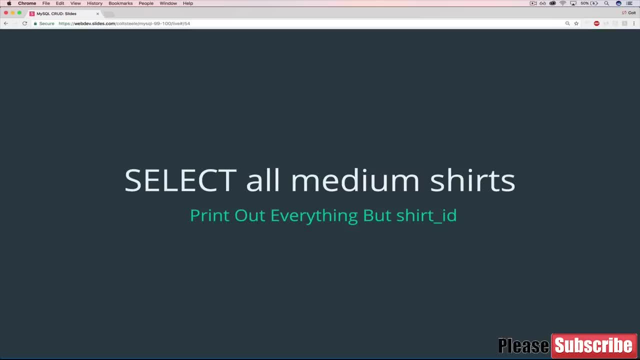 which excluded shirt ID. Sorry, shirt ID. So that's it for the selecting portion. the read in our crud Next up update. So we've covered creating and reading. Now we're on to updating our shirts. So the first problem is to update all polo shirts. 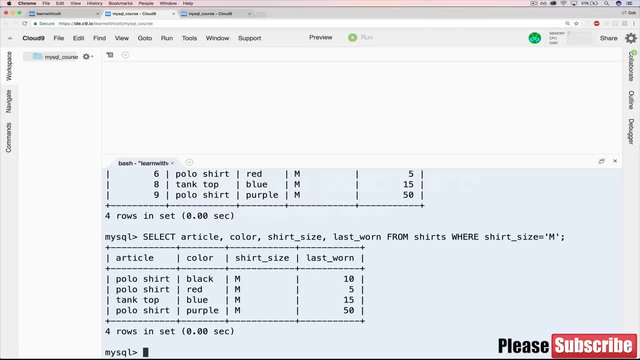 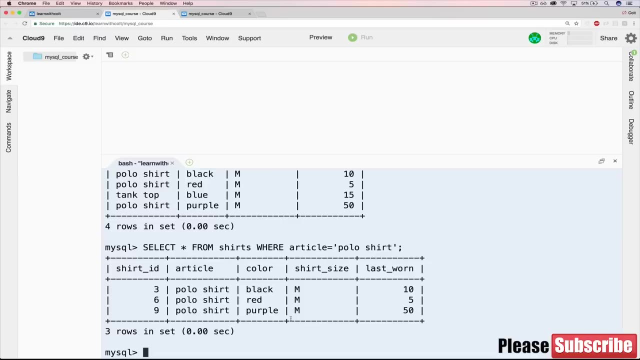 and change their size to be large. So we'll start by just selecting polo shirts. Select star from shirts where article equals polo shirt, Just like that. Okay, So this is what we get, And what we want to do is change shirt size to be large. 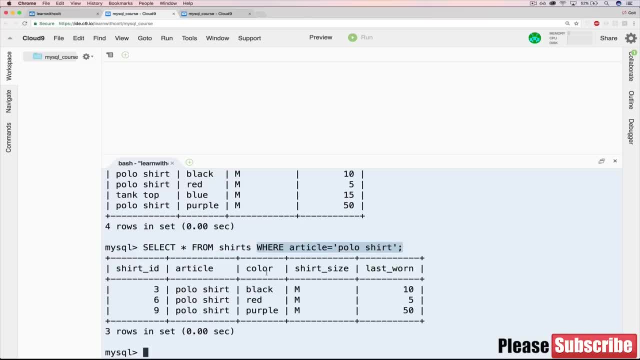 So we need to keep this. I'll copy it now And then we'll type out: update: shirts set And we want to change shirt size to now be large. And where do we want to do that? Only where article is polo shirt. 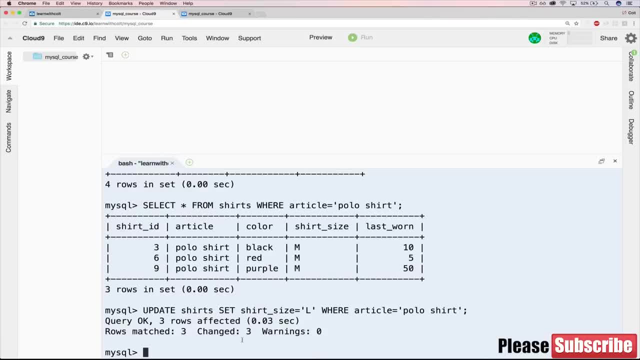 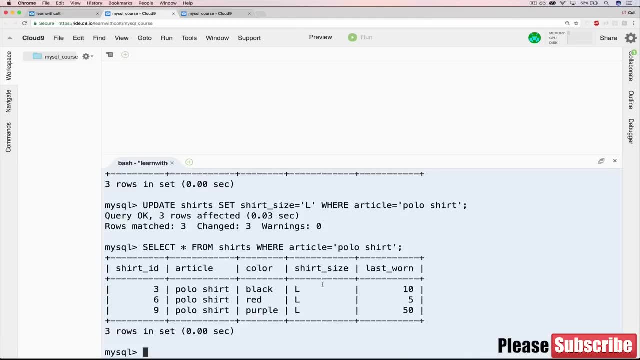 Hit enter, We get three rows affected, three rows changed. Now if we go back and run our same select, we should see all polo shirts are now larges. We can do the same thing, Just to see it in the grand scheme of things. 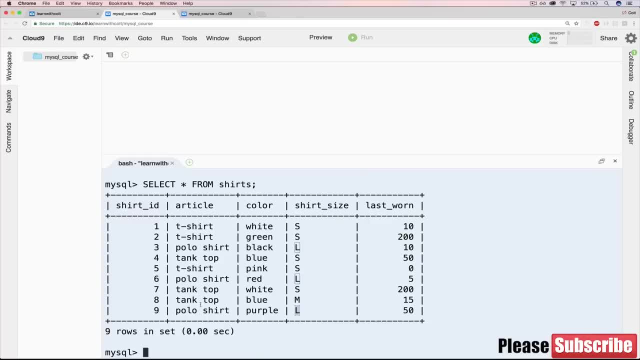 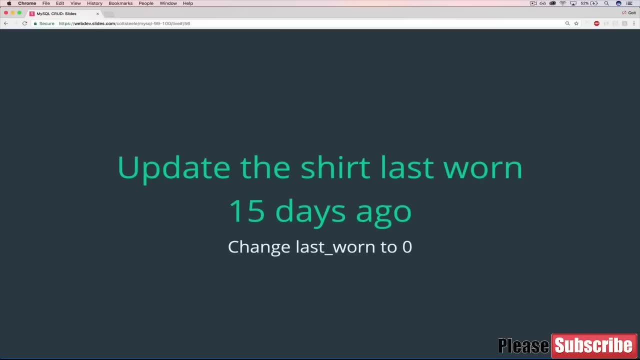 There we go. We have three larges now, All polo shirts. The next problem is to update the shirt last worn 15 days ago and change last worn to be zero. So we'll start by just selecting that shirt, like we did earlier. 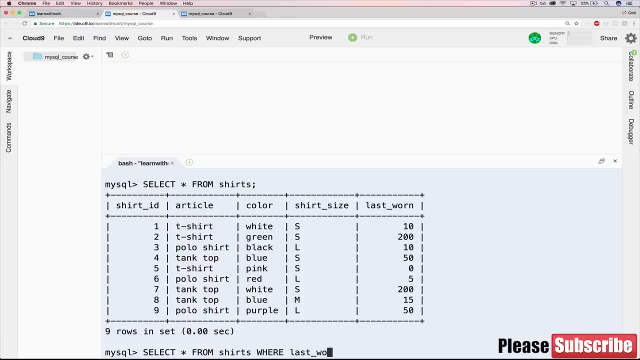 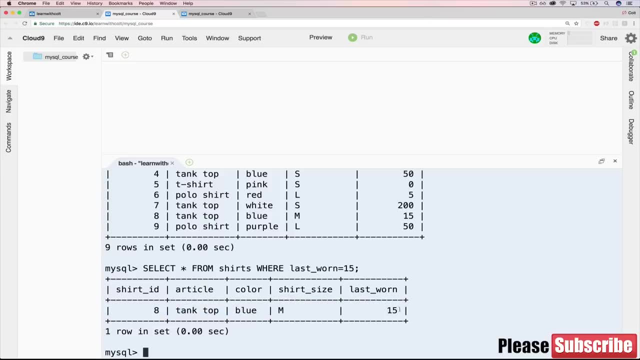 Where last worn equals 15.. There it is: Tank top, blue, medium, last worn 15 days ago And we wore it. We wore it today. It was a hot day, We needed a tank top And we want to update last worn to be zero. 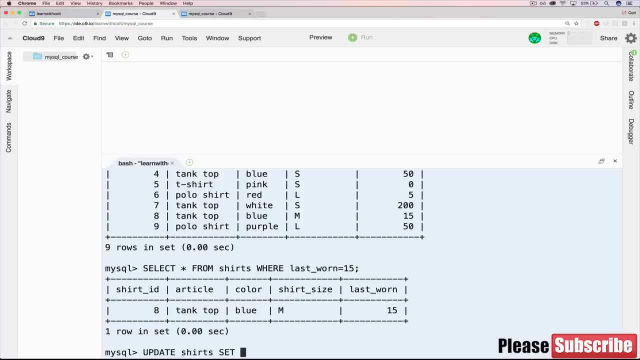 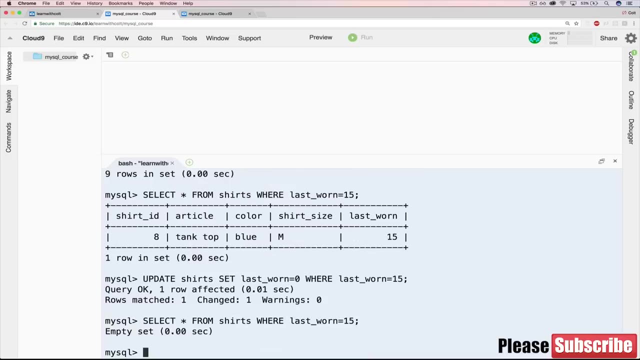 So update shirts set last worn equal to zero Where last worn is currently 15.. We get one row affected, one changed. Let's do our select again. We no longer have it. But now, if we say select where last worn is zero, 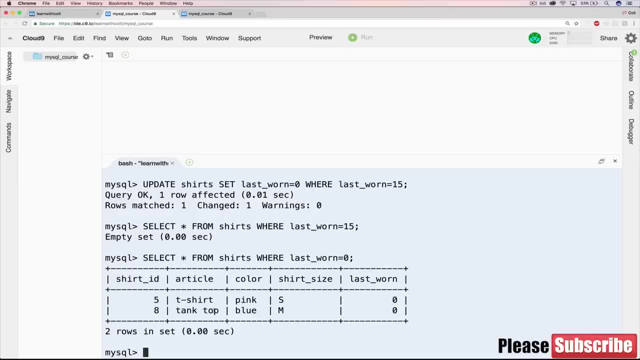 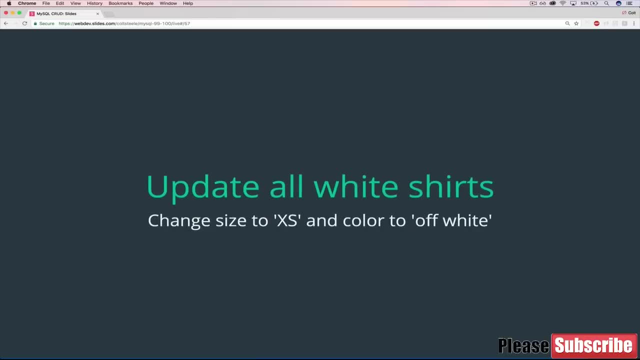 we have two shirts: This t-shirt that was already there and our blue tank top we just added- Perfect. So the final update is to update all white shirts, change their size to extra small and, at the same time, change their color to off-white. 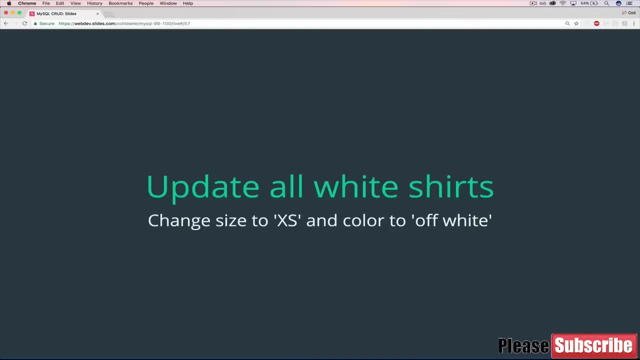 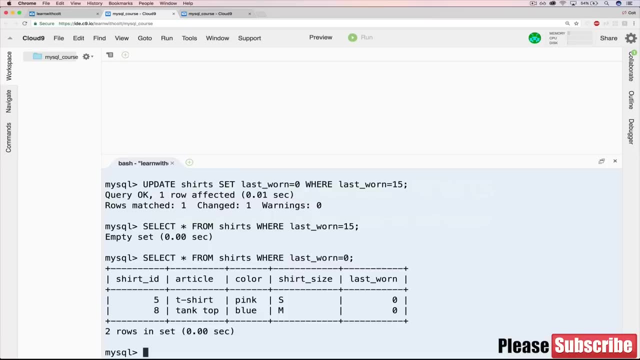 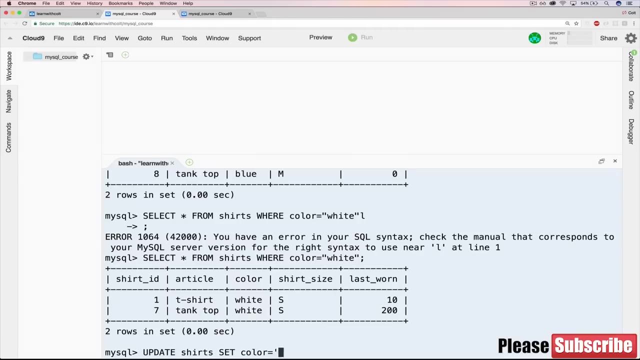 So this needs to happen all at once. You can't do two lines. I mean you could, but that's against the rules for this problem. So let's start off by just selecting all white shirts. Select star from shirts where color equals white. 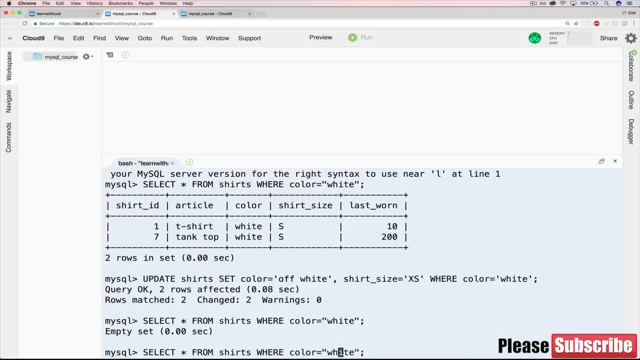 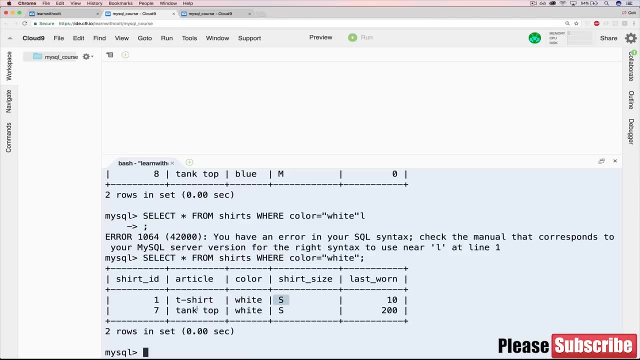 Oh boy, Let's get rid of that extra L there. Here we go. So we have two shirts: A t-shirt that's white, that's small, And a tank top that's white, that's small. So we want to change color to be off-white, and shirt size to be extra small. 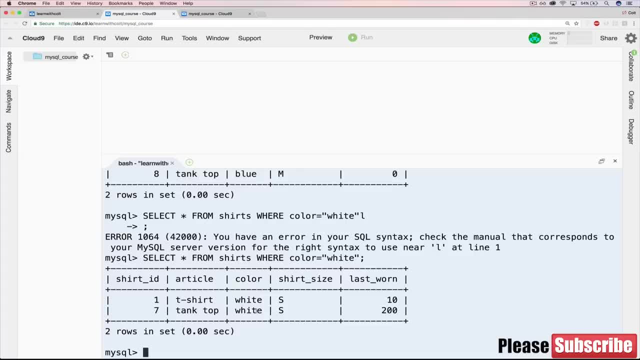 because we shrank them and we mixed them with colored stuff in the washing machine, so their color is now off-white. So to do that, let's start with the first part- Update shirts, and we'll set color to be off-white, And then we'll do the second part with a comma. 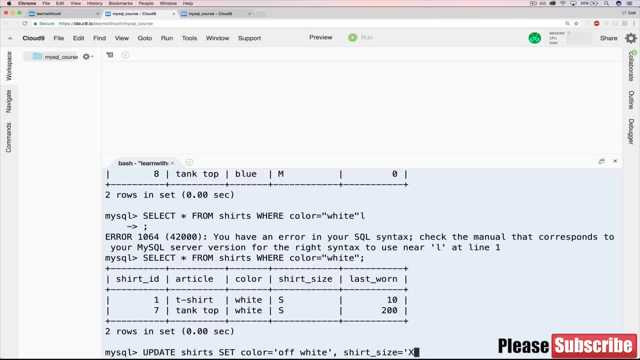 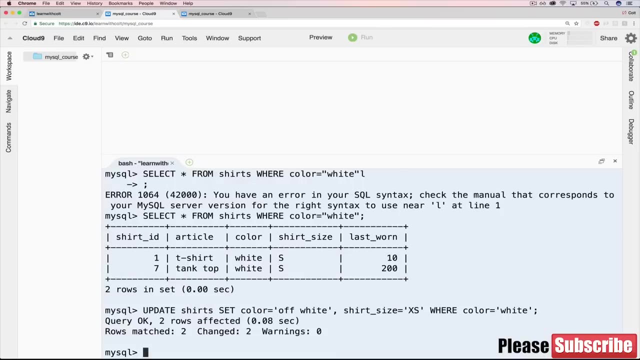 Shirt size equals XS: extra small, Just like that. And then we'll do our where color currently equals white, And that should do it. Fingers crossed, No typos. Now, if we go back and select where color is white, we should have nothing. 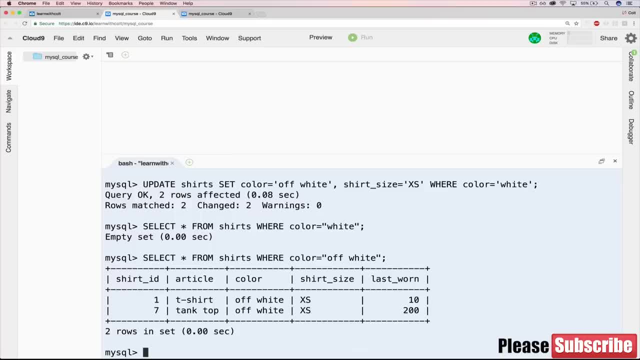 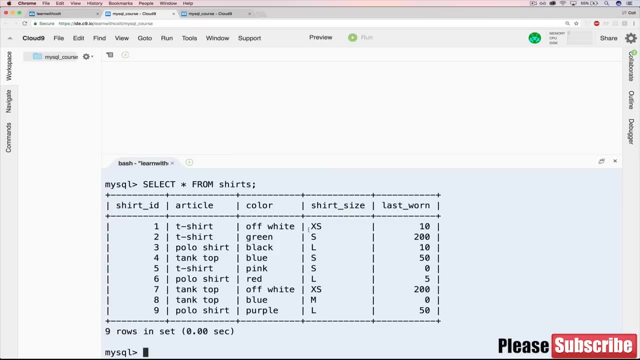 But if we say where color is off-white, we should have two that are extra smalls, or we could, of course, do select star from shirts. to check our work. We have extra small off-white, extra small off-white. Okay, So that problem was just making sure that you could update multiple fields at once. 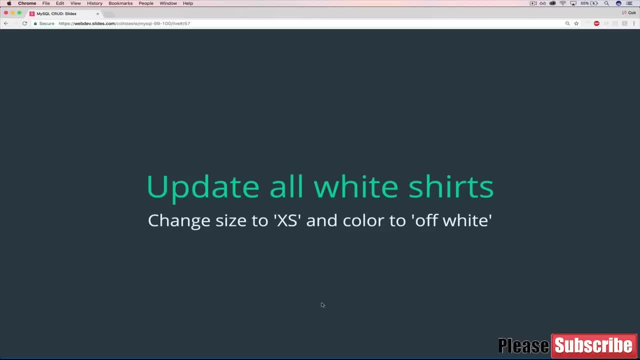 making sure you understood that. Okay, That's it for update. Next we move on to D- delete. Okay, So we've made it to the end. the final video solution to our spring cleaning extravaganza problem. Now we need to delete. 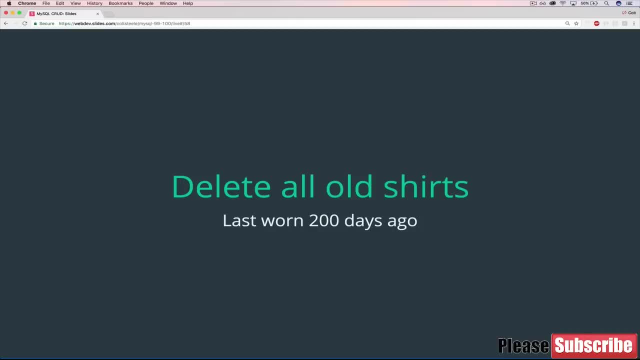 We've covered creating, reading and updating, basically inserting, selecting and update. Now we're going to use delete. So the first thing is to delete all old shirts, which really, just in this case, means last worn is 200 exactly. 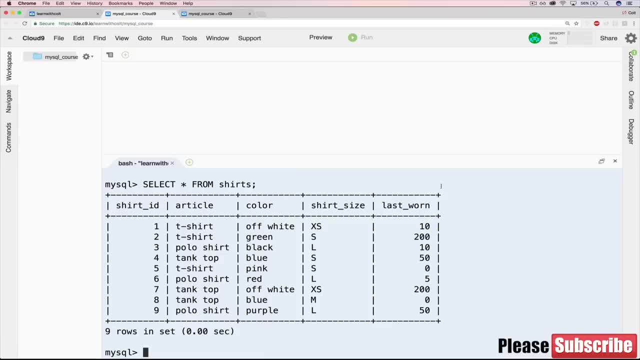 So when we do our select star, you can see there's two shirts that meet that criteria: 7,, ID of 7, and ID of 2.. But we're going to delete them based off of last worn. So we always start with our select star from shirts where last worn equals 200.. 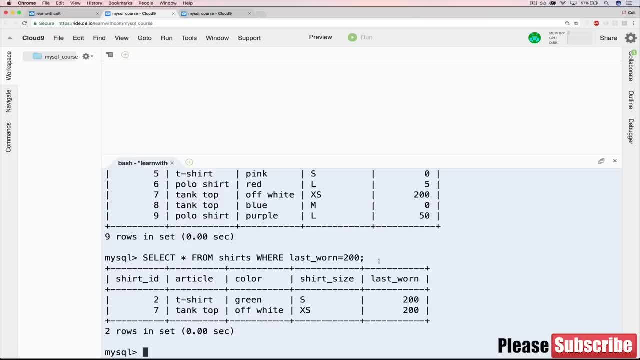 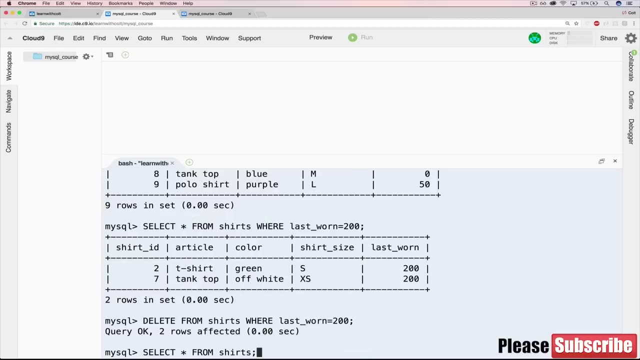 And we get our two shirts, So then we can copy this And actually we can copy this entire thing. Delete from shirts where last worn is 200.. Two rows affected. Now if we do a select star, those two are gone. You can see it goes from 1 to 3 and then from 6 to 8.. 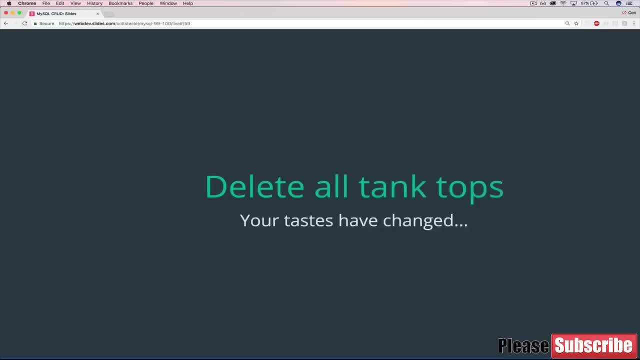 And there we go. So the next problem is to delete all tank tops. We've decided tank tops make us look kind of stupid, So we're going to delete tank tops. So your tastes have changed. So how many tank tops do we have? 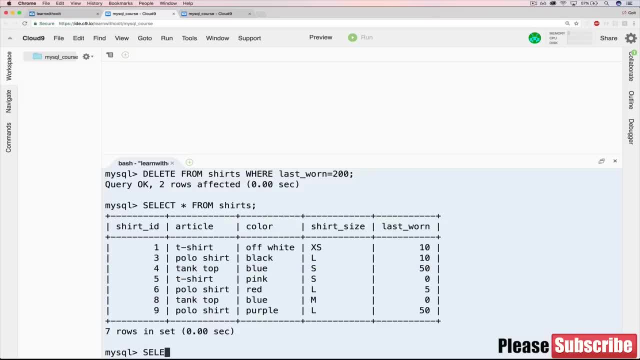 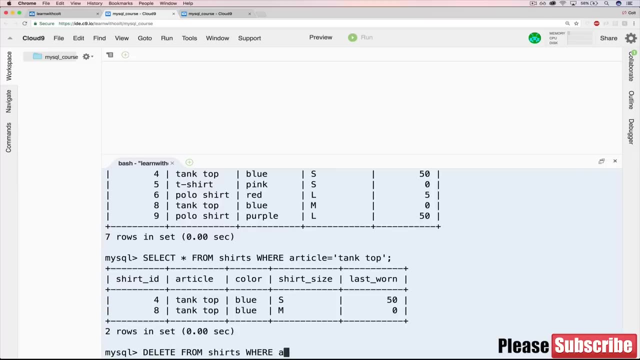 We've got 1 and 2 that are left, So we'll do a select star from shirts where article equals tank top. We get 2. Then all we need to do now is delete from shirts where article equals tank top. Hit enter. 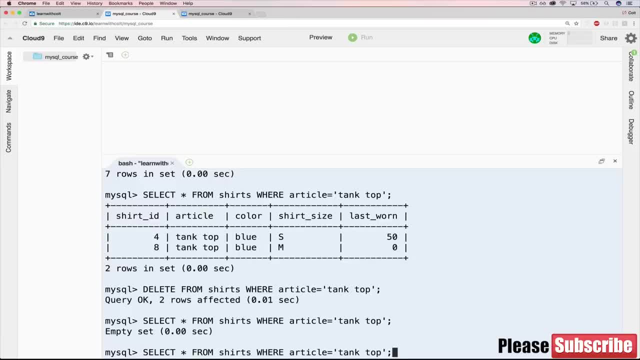 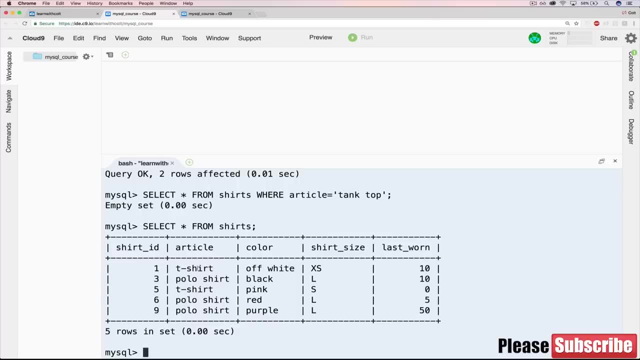 Now, if we try and select them, they're gone. And if we do a select star from shirts with no wear clause, now we have 1,, 3,, 5,, 6,, 9.. So we've lost our two tank tops. 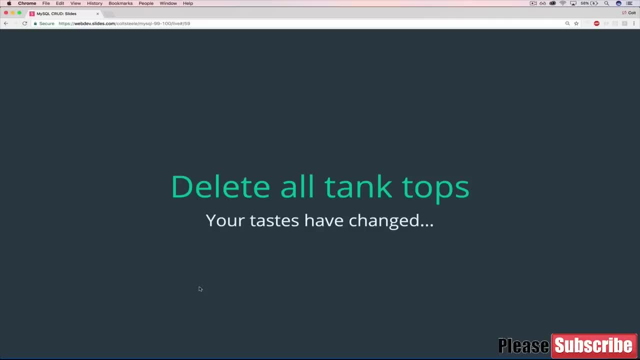 All we have are t-shirts and polo shirts, which leads us to our final exercise here: Delete all the shirts- And I lied, It's actually the second to last. So to delete all the shirts, but not the entire table. it's pretty simple. 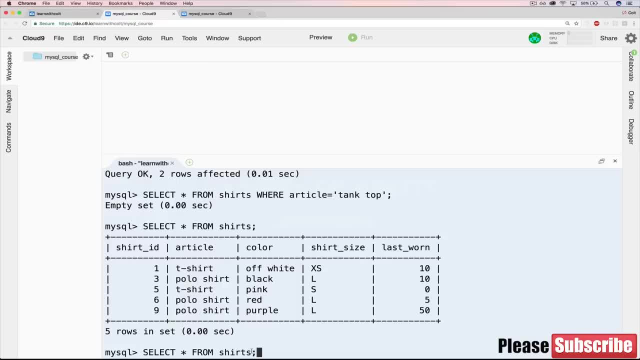 We use the same wear clause, which is to say that we don't have a wear clause. So in this case it returns select star from shirts, returns all shirts. Well, we just replace that Delete from shirts, if I can spell it correctly, with this part. 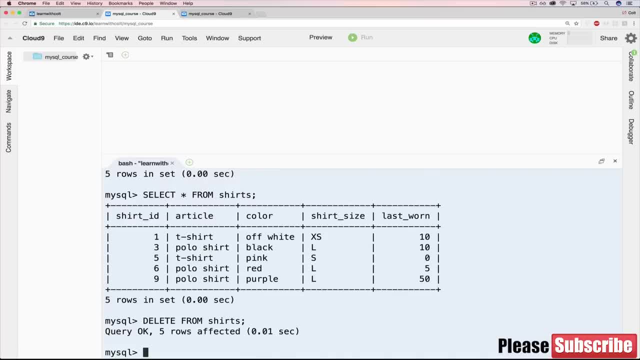 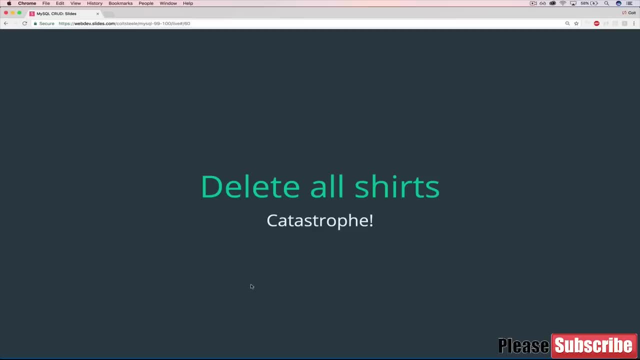 And, moment of truth, 5 rows affected. Now, when we do select star from shirts, we get nothing. It's a sad day- Not as sad as when we deleted the cats, but still sad- And the last thing is to drop the entire table. 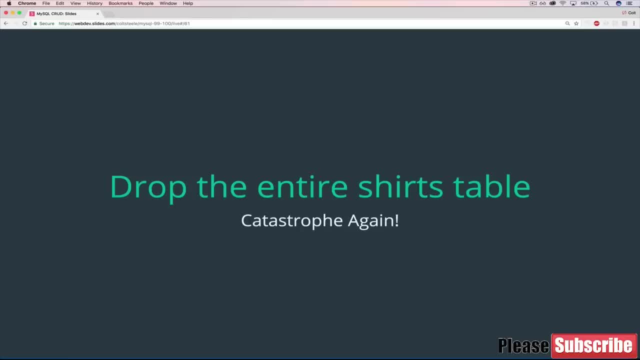 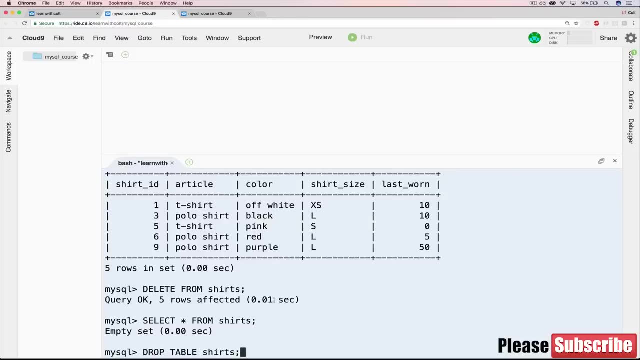 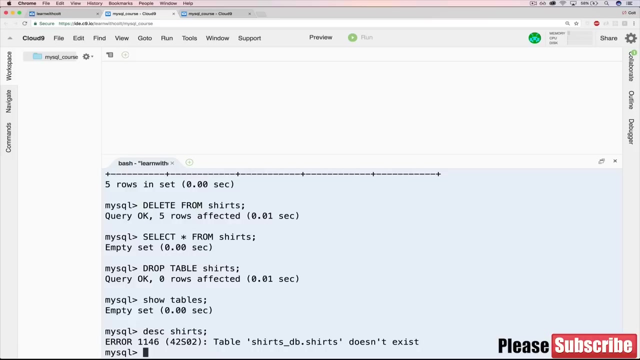 We're just done with this. We hated this exercise. We want to move on. So drop table shirts. Now hit enter. And if I do show tables- no tables. And if I try and describe shirts, we get an error because there is no shirts table to describe and it freaks out. 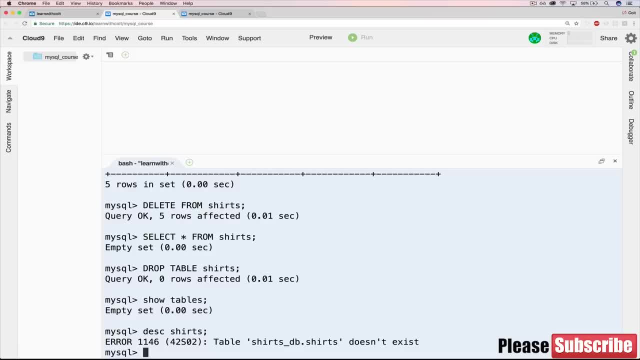 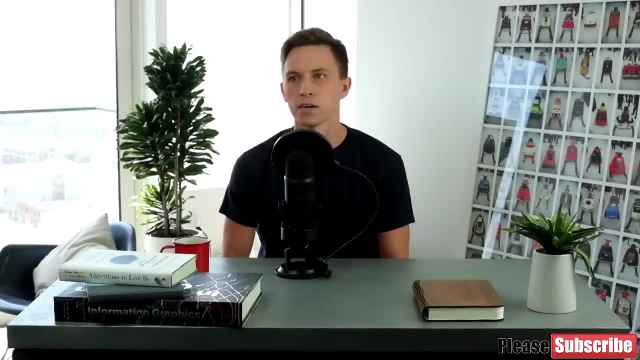 So we've successfully deleted it. Now we have an empty database that we don't need anymore, And we're done with this, Congratulations, Hey, welcome to another one of these videos at the beginning of a section where I just make a fool of myself and do something ridiculous. 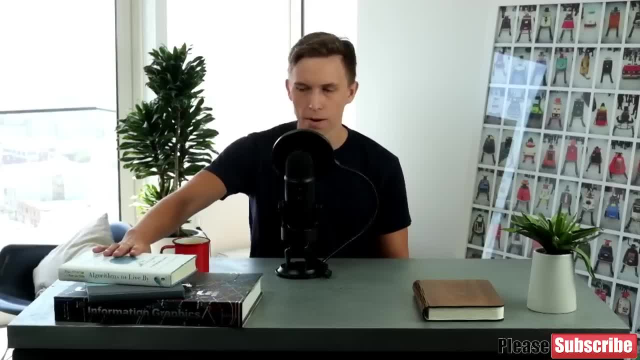 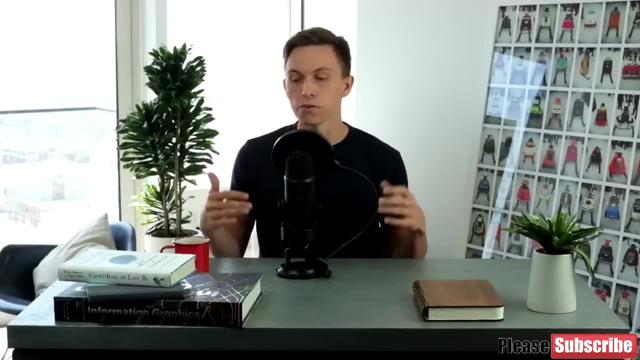 This time we're working with books. As you can see, it got more props- Just really love props- on this course- And they're here for a reason: because in this section we're getting introduced to our new data set. So for the next couple of sections, we're going to be working with one data set that I'm going to give you. 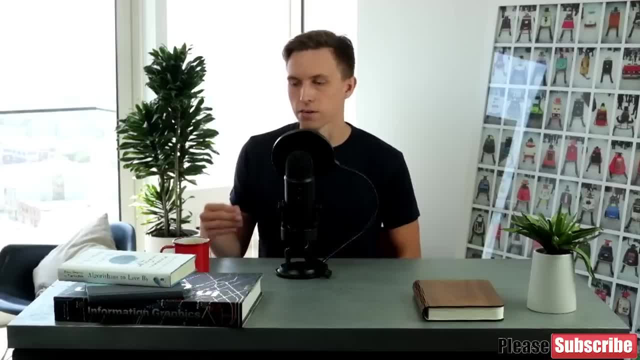 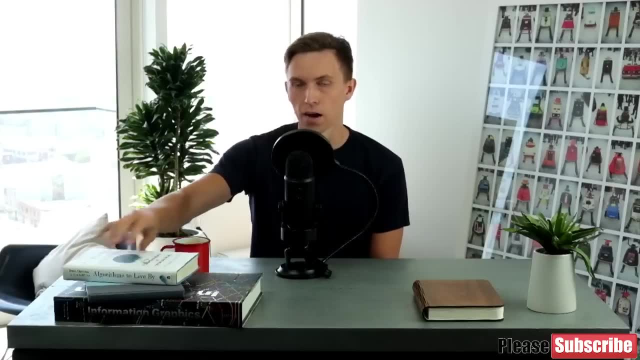 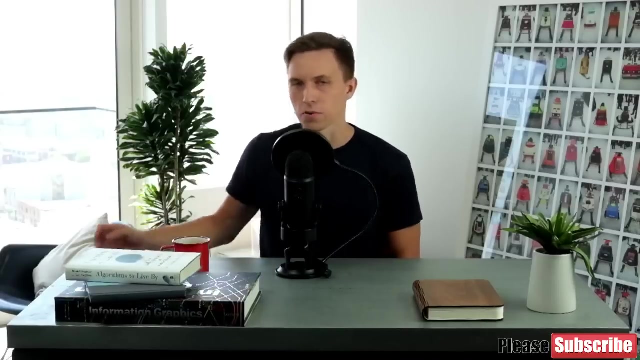 And it has to do with books, And books make a particularly good data set because there's a lot of data to model. We've got things like, you know, titles, genre, the authors, how many authors there are, things like reviews, ratings, page count, release dates, tons of information for all different sizes of books: giant, prop books, medium, small books, all that fun stuff. 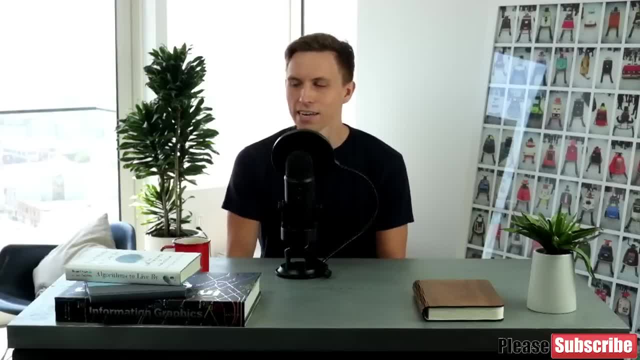 And our back story here is a very weak back story. We run a small online bookstore and we're being just slaughtered by Amazon, So we're fighting back the only way we know how, which is redoing our database inventory management system. So that's what we're going to do. 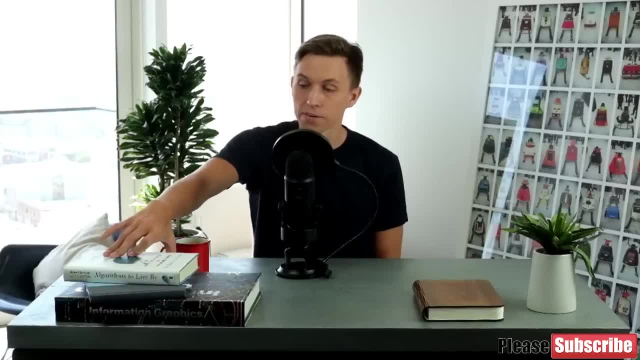 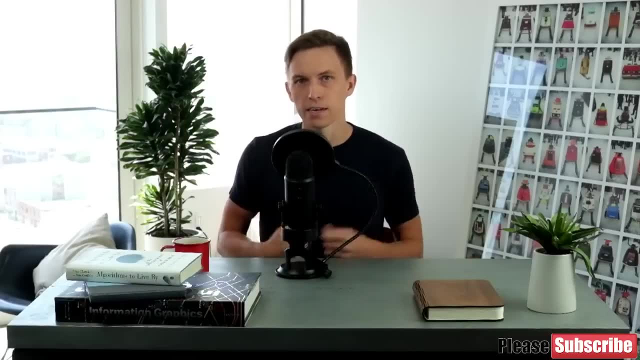 We're going to fight back by redoing our database, and that will be what we start this section doing. But then, once we have that data in the database, we're going to move on to learning a bunch of new commands, And those commands all are called string functions. 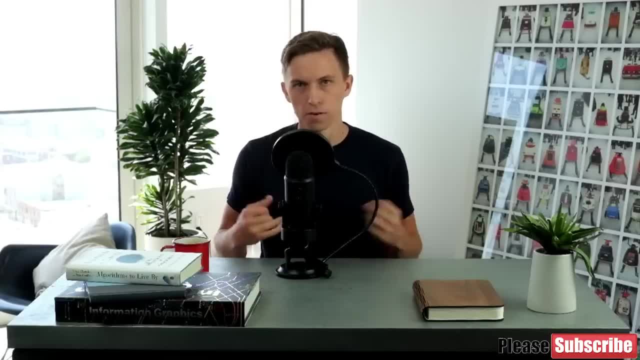 So I'll explain what those mean in just a little bit. I don't want to make this video too long, But basically they expand our way of selecting data and working with text or with strings- really important and kind of fun things that we can do. 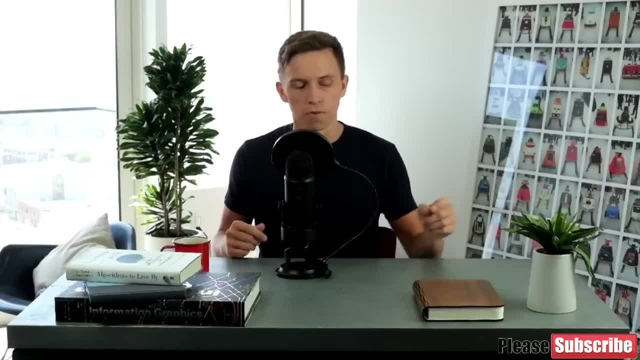 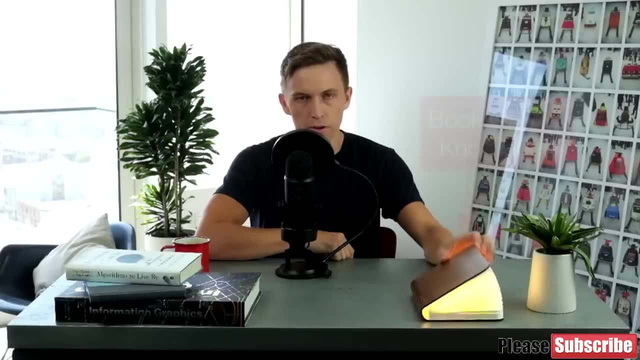 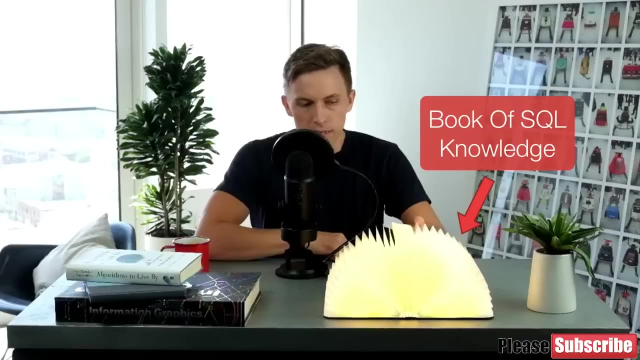 So we're going to go ahead and get started. Oh, before I forget this book, here is a very important book. This represents the book of SQL knowledge. Yeah, kind of regret this now, but this is the book of SQL knowledge. 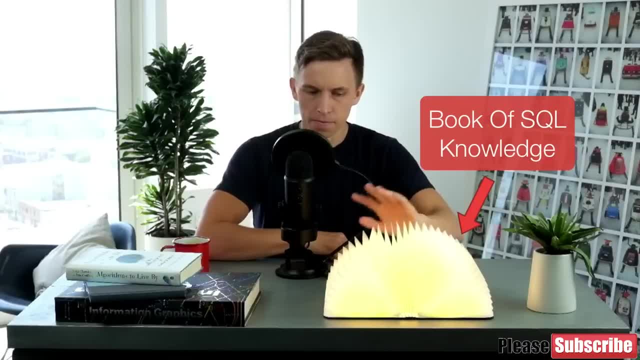 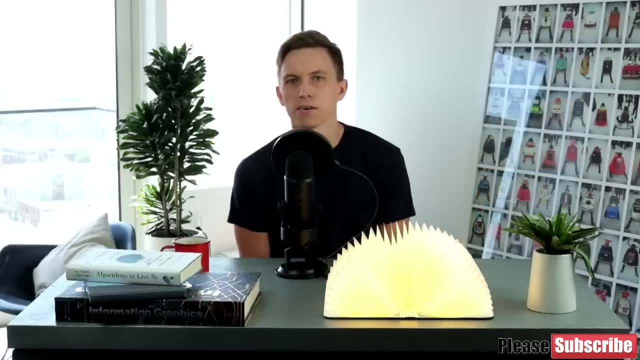 You can ignore. There's a bunch of bugs in here. They're attracted to the light. You can ignore that part. Our book of SQL knowledge doesn't have any bugs in it. We are bug free. Anyways, I think I should probably end it here. 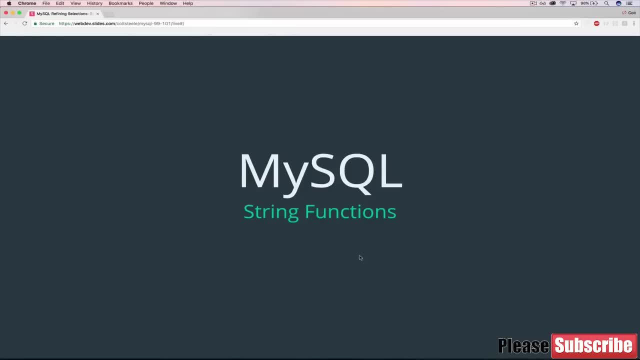 I'll see you in the next video. Okay, so we made it through all of that crud. That's sort of a joke. Anyways, we're now talking about string functions. So basically, we've seen how to interact with our database: create stuff, insert it, update, delete. all of that. 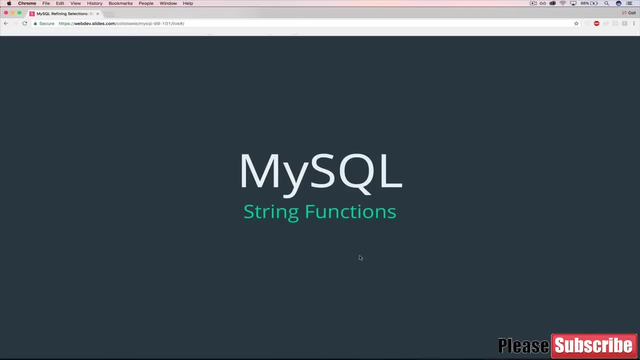 But now we're going to focus more on select Or reading the data out, Because what we've been doing right now is just reading the data directly as it is. So I could say: you know, I select breed and name from cats. 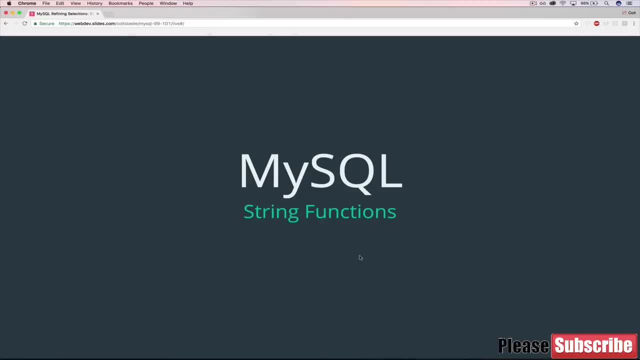 And that's it. I get it back And that's great. But there are things that I could do with that data. So with numbers, I might want to add them together, Or I might want to- I don't know- reverse a string or replace all spaces with a certain character. 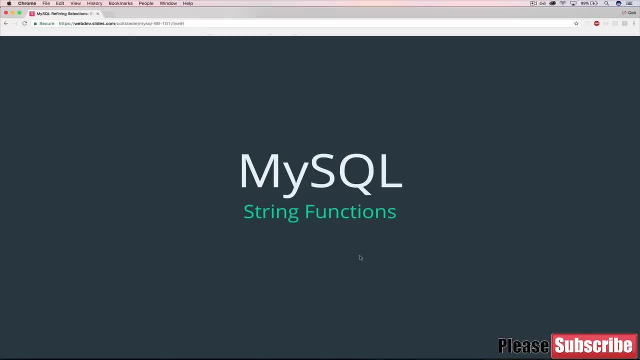 Or conjoin- first name and last name Or conjoin- you know two pieces of data. You know two pieces of data together. All of these are different operations, different ways of printing our data out that we can do, And so we're going to start focusing on them in this section. 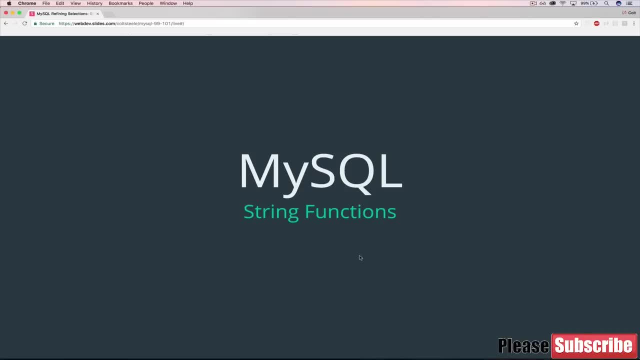 We're talking about string functions, So there's going to be a bunch of things that we see. I already mentioned some of them. We can concatenate words. We can take certain parts of a string and leave other parts out. We can reverse. 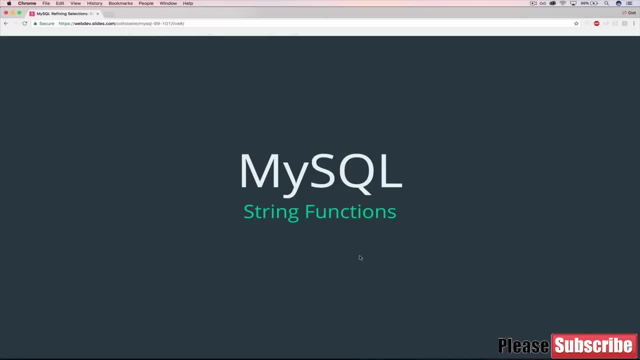 We can uppercase, lowercase, replace characters, all sorts of things, But before we get there, The first thing I want to do is show you Something that I think is pretty useful and that we'll use pretty often from here on out. So up until this point, all of the SQL that we've been writing has been manually entered into the command line, into the CLI here. 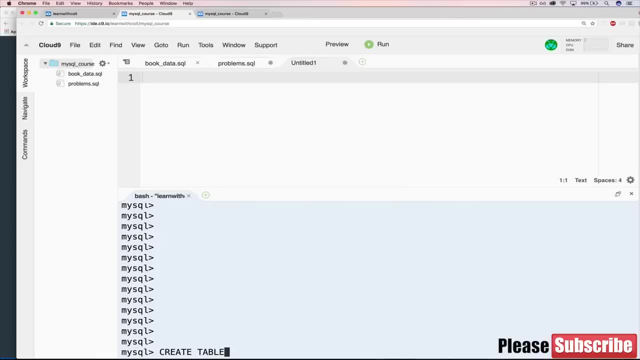 So if I want to create a table, I have to type create table and then the name of the table: cats. But let's say that I mess it up. So let's say I typed singular cat, which technically isn't a problem per se. 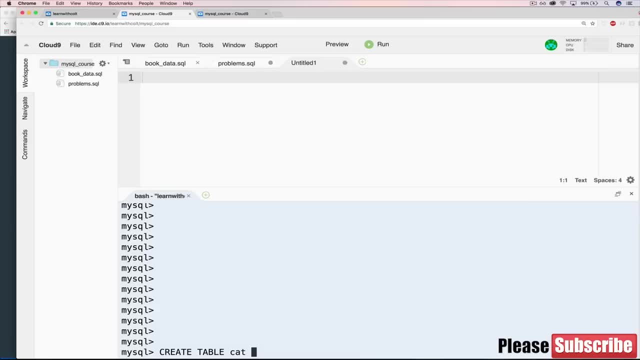 But it's a good idea to have things pluralized. It won't break. But so let's say I don't notice for a little bit though. So I create a table cat and we want you know name is Varchar 100.. 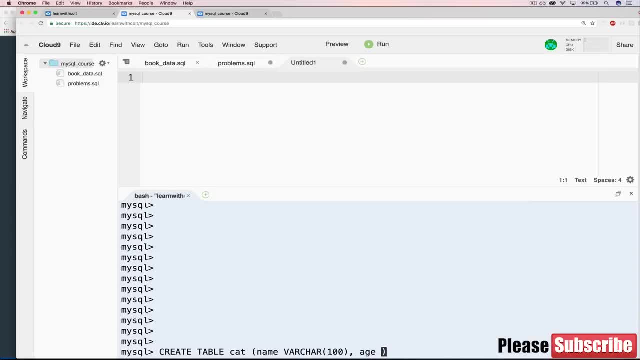 Age is 10.. What am I doing? Age is int, Just like that. Let's say we leave it at that. Now, this isn't a great example, because this is a short line, But if I messed it up, I have to go all the way back here and edit it. 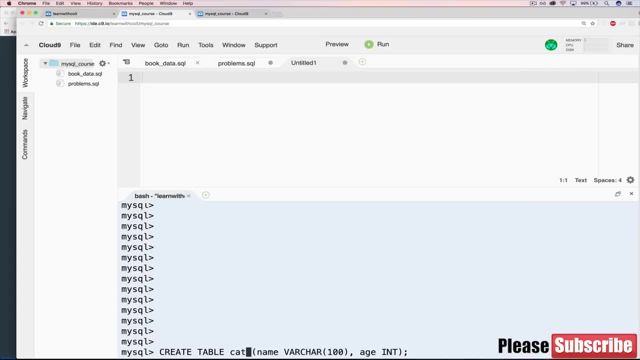 Right And do cats Like this. But let's now suppose that I have something even longer and I want to put it on separate lines and format it nicely, like this Great table cats. And then we have parentheses there and we'll do. name is Varchar. 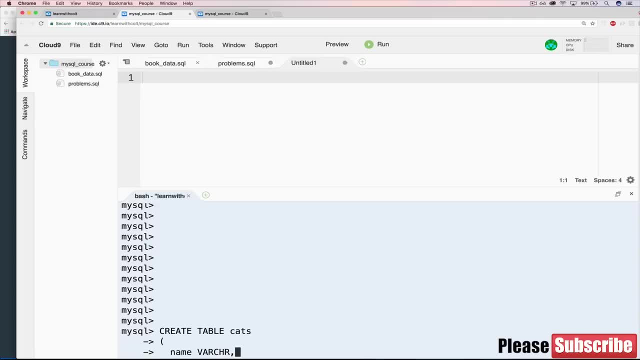 And let's say I misspell this like that, And age is an int. And then I realize, oh shoot, I totally messed up. I don't have a way of getting back there. I don't have an easy way of getting here. 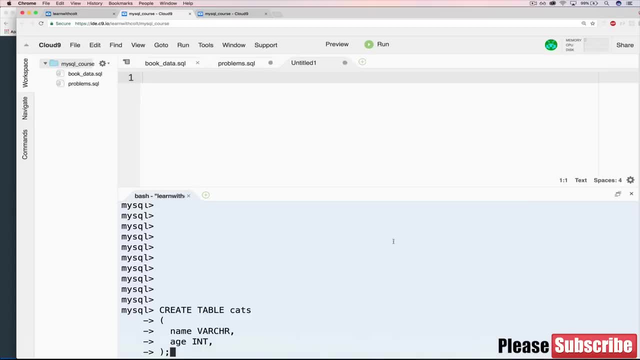 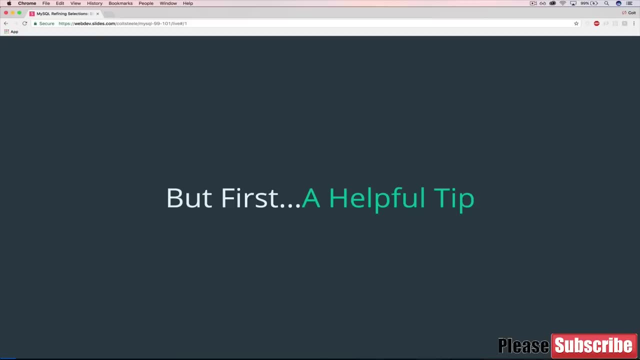 So I have to retype the whole line or copy it. There's no simple way of editing it. So what I want to show you is that we can run code from a file, And that's really, really useful. Running SQL files. 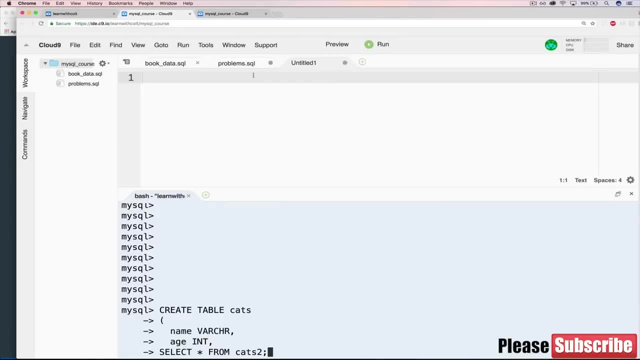 That's what we're going to talk about here. So basically, by the end we will be working with files that look like this: They're nicely formatted, They have nice syntax highlighting, We can edit them, make changes and so on. 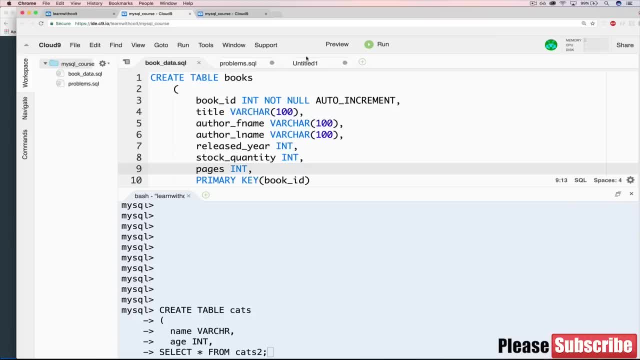 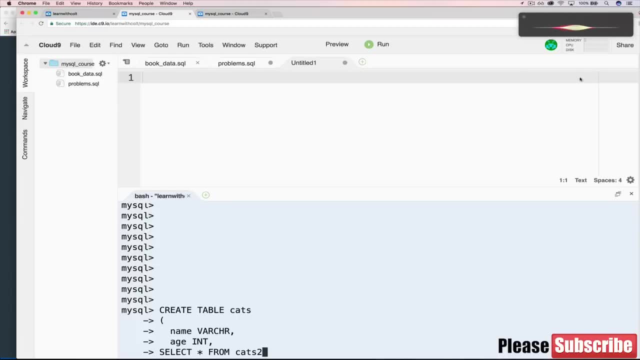 And run them when we're ready, rather than typing things manually into the command line. That doesn't mean that we won't be typing things here, because it's a very useful tool. Oh, go away, Siri. It's a very useful tool. 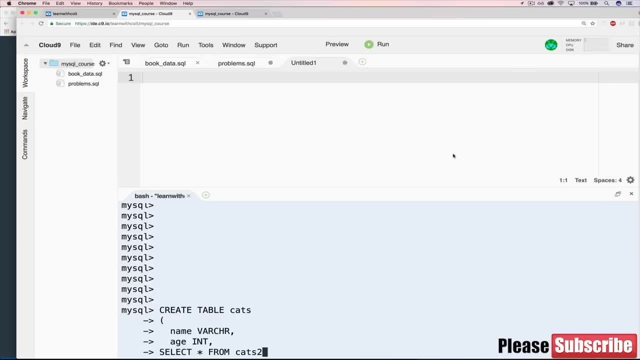 I should probably edit that out. Anyways, it's a useful tool that allows us to explore things, try things out. If they're short lines, it's great, But if we're really trying to do more serious stuff, it's much easier and better to work in a file. 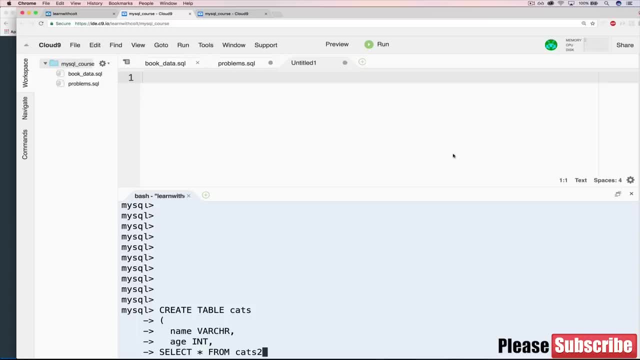 You can make edits, You can share it with people, So that's what we're going to do. So let's go ahead, Let me get out of this And I'll just hit enter and get an error, And that's fine. 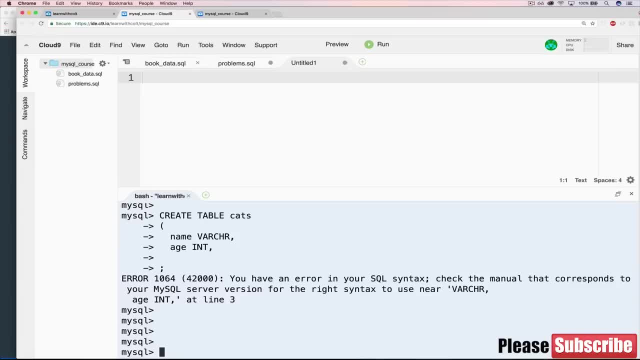 So right now I'm in cat's database And if I do show tables, we don't. Oh, I do have a cat's table, But if I look at it it's empty. So what I'm actually going to do is drop that cat's table. 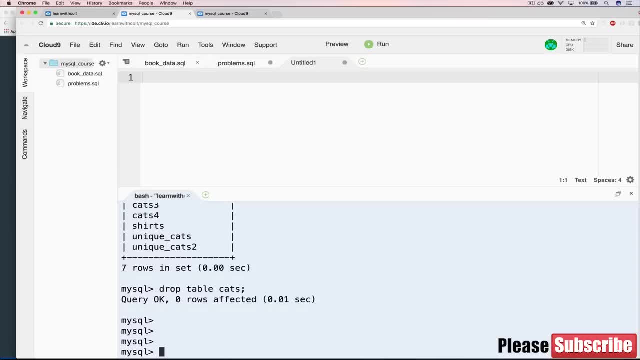 Drop table cats. Okay, So what I want to do is remake the cat's table, And what I could do is what I just did here: Create table cats and do the whole thing. But rather than that, I'm going to do it in a file. 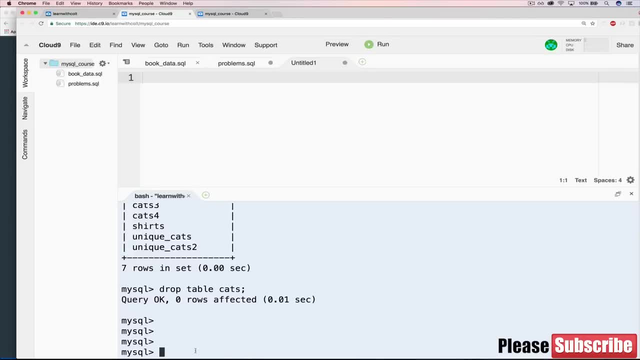 And then all I'll have to do here is run that file. I'll execute it with one short line. So up here I have a new file. Again, you can do file new file. You can use the shortcut shown here. 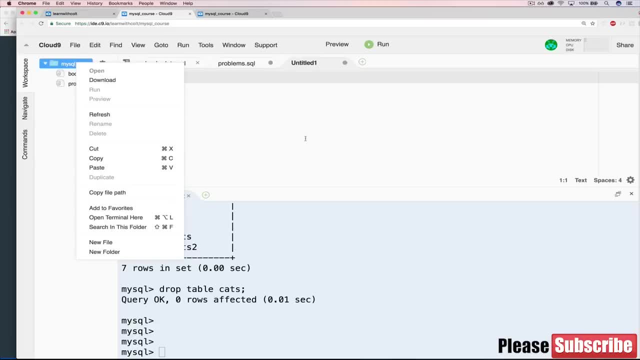 You can right click and do new file as well. Whatever we do, though, we need a new file, And I'm just going to put something in there, So create table, And I am showing you creating a table, But we'll be putting any SQL query in here. 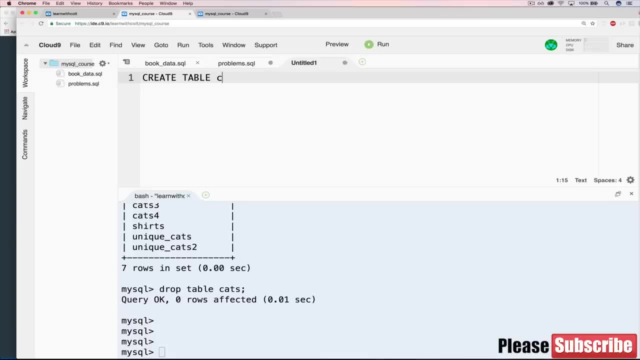 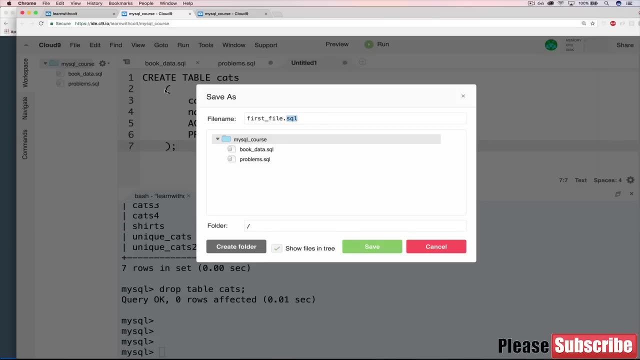 Creating a table, dropping tables, inserting data, selecting any sort of query we want. So create table cats. And it's so easy now to format it nicely. We'll have name which is varchar100.. Let's do an ID as well. 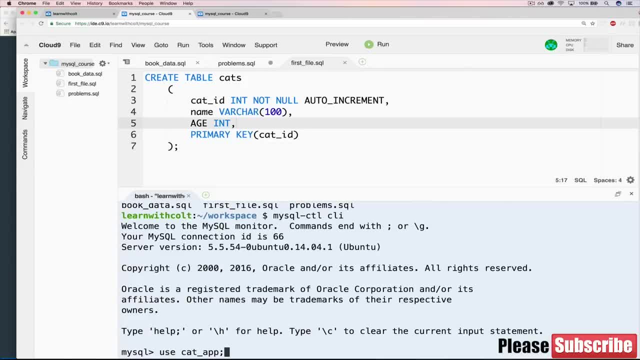 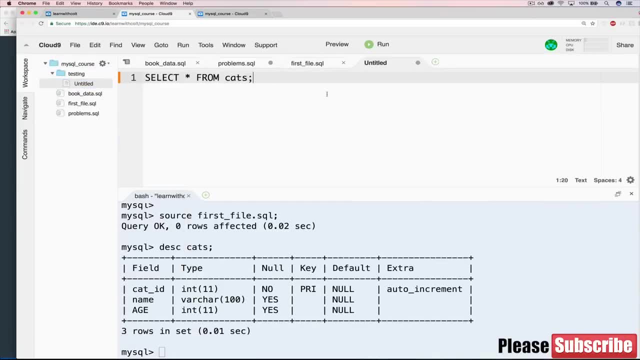 See how easy that was. if I made a mistake, Cat ID will be an int, not null auto increment, comma, name, varchar, And then we'll do age as an int And we'll do primary key is cat ID. 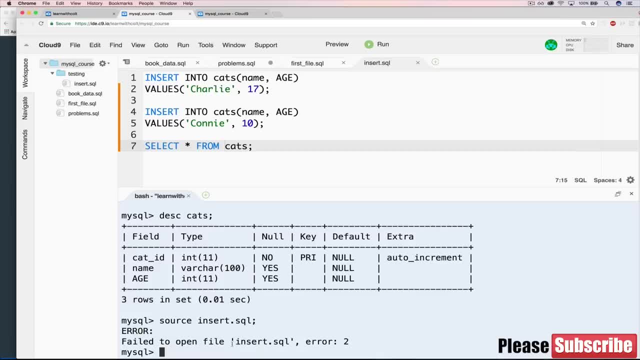 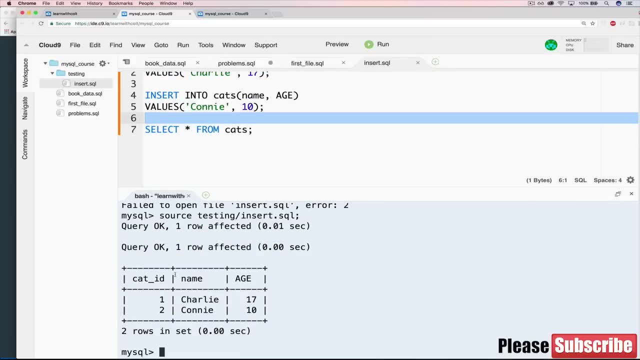 So this should all be review. But what's nice is I have this query like this: I need to save the file, So I did command S, but you can also go file save And we need to give it a name. Any name will do. 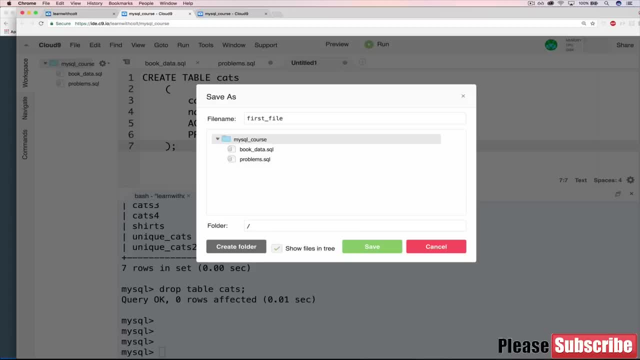 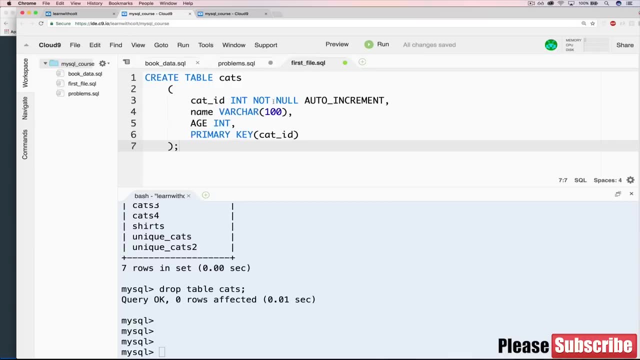 I'll just call it first file, And this is the most important part- sql. So that's what identifies the contents of the file as SQL code. So we need that. Click save. Make sure it changed up there Also. you can see we got nice syntax highlighting now, which is also very useful. 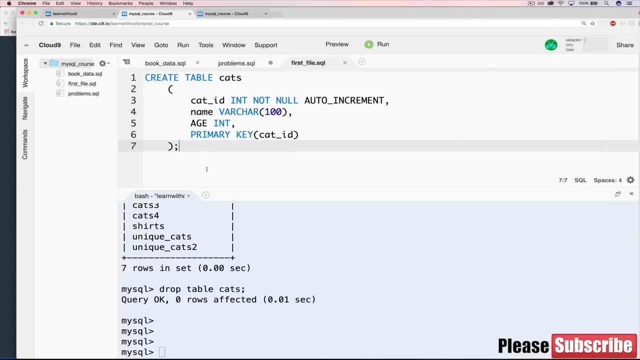 Okay, So I'm sure by now you can see the value in doing this. You have a history of your work. You can edit it, share it with people. It's just a much better way of doing it. So how do we actually run it? 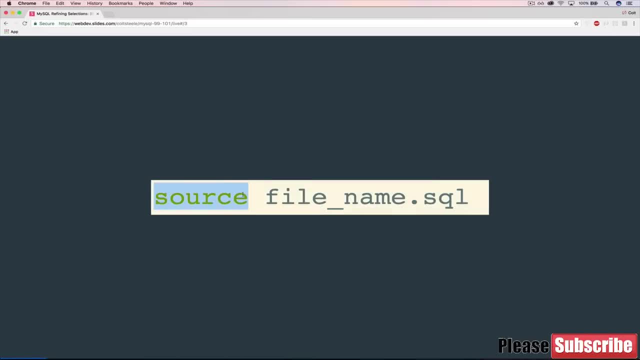 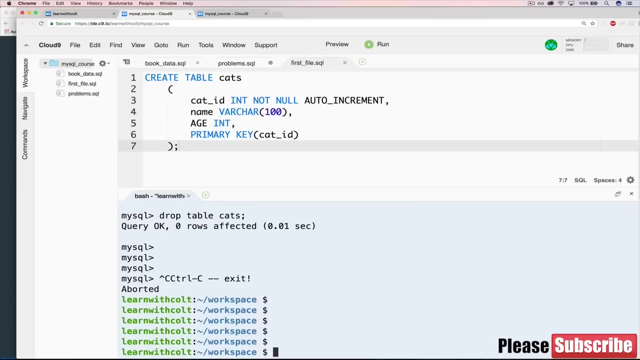 Well, this is the magic Source and then a file name. So in our case, our file name is first file sql, So we just need source file name sql. So I'm going to actually quit out of the CLI And the first thing I want to show you is that it matters where you are when you initialize your CLI. 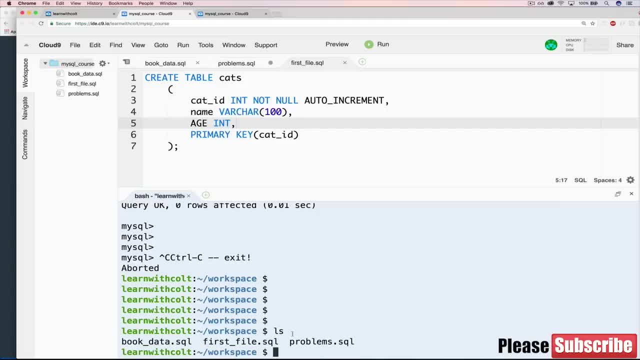 So when I type LS here- and if you're not familiar with that- it just lists the current files. So what this shows me is that I have book data first file and problems All right. So we want first file, Don't worry about these other two. 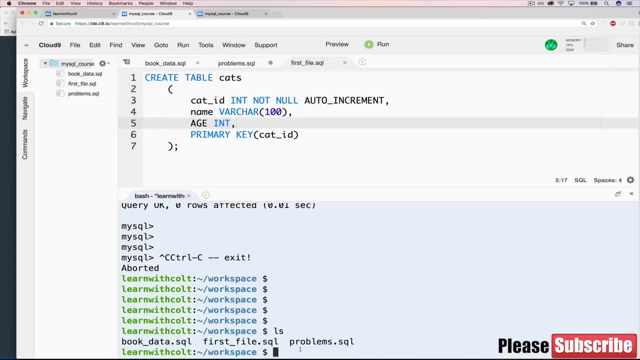 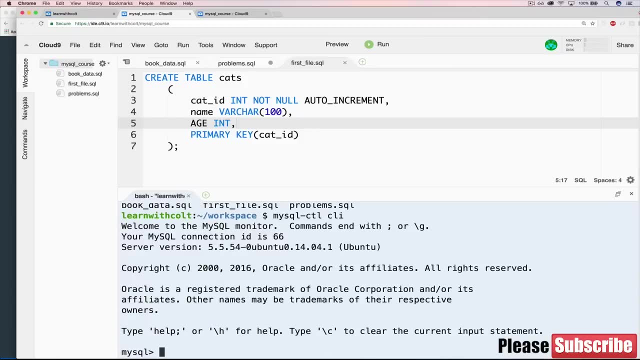 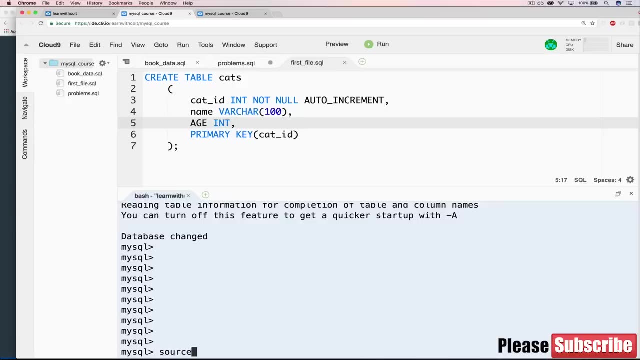 So we are in the correct directory to access that file. So if I start up the CLI with mysqlctl CLI And I use the cat app database, Just like that, I'll make some space. Now all I have to do is source first file sql. 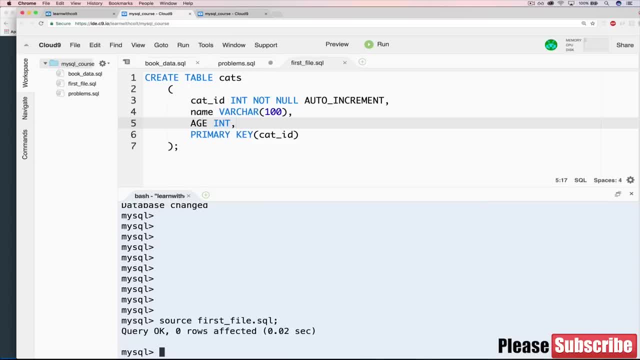 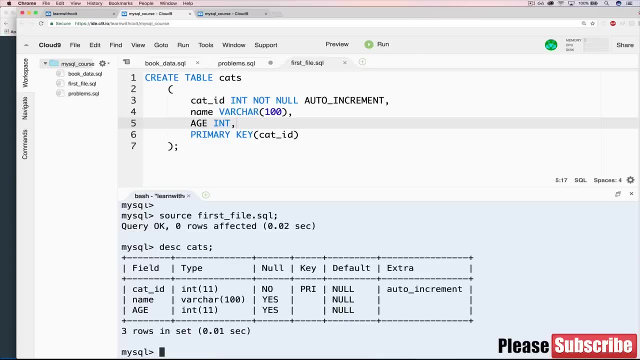 Just like that And we'll see what happens. It says query- okay. So now how do we know what works? Well, we could do a describe cats And here's our table. So that's all that there is to actually executing the file. 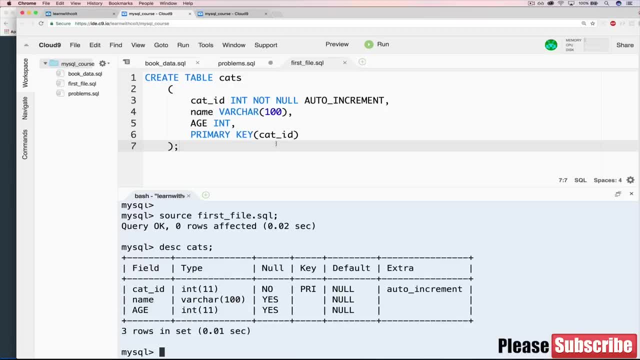 It's just the source and the file name. But what I want to show you two things. I'll go ahead and make a new directory. You don't have to do this, But I'm just going to call it. I don't know. testing. 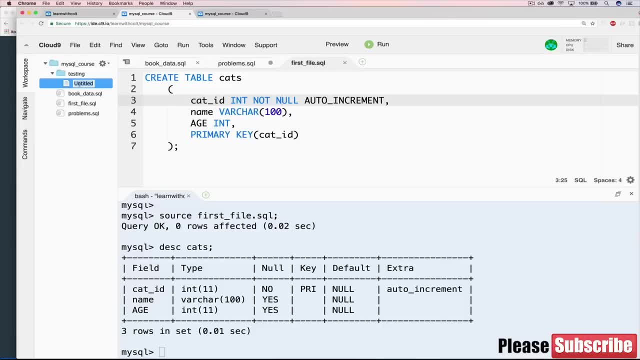 And then, instead of testing, I'll make a new file And what I'll put inside of that file is a select statement, Select star from cats. Actually, let's do an insert, Insert into cats, And we'll just do. what do we have here? 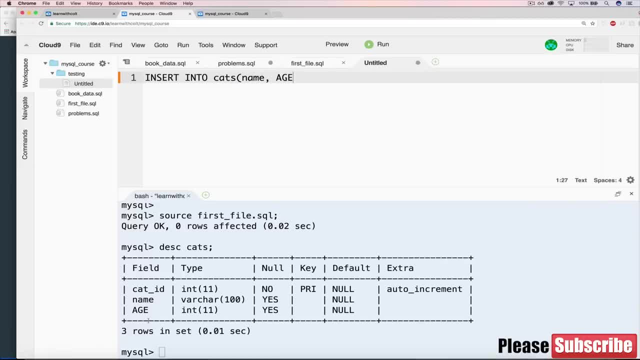 Name and age which I'm just realizing I capitalized, So we could obviously go back and change that here and rerun it, But we'll leave it. So insert into cats name, Name and age, just like that Values and name will be. let's do Charlie. 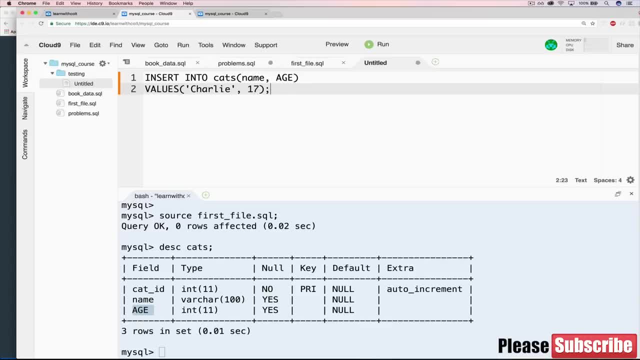 And age will be. let's do an old cat 17.. Save the file And we'll do file save And make sure the file has sql in it. So we'll do rename And I'll just call this insertsql. 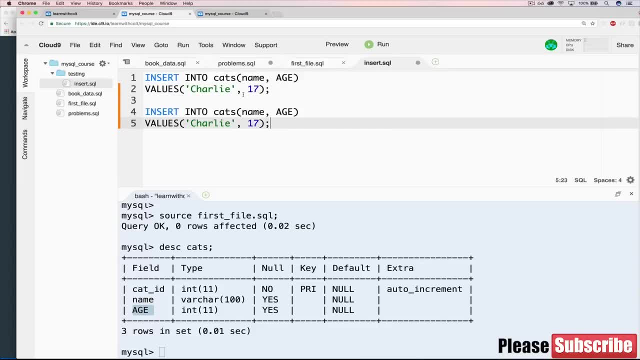 Okay, Let's actually just to show you we can do more than one thing at a time. let's insert both, or let's insert two, And this one will be called. I think we already have a Cindy. Let's do a Connie who is 10.. 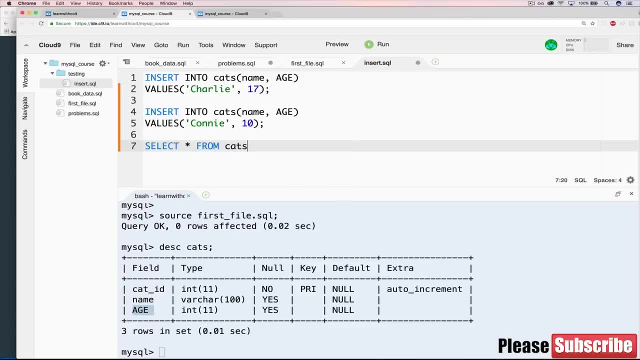 And then at the end we'll also do select star from cats, just like that. So these three things will be executed at once if we do it correctly. So now to reference this file: Our CLI is running in this folder, So we can't just say insertsql. 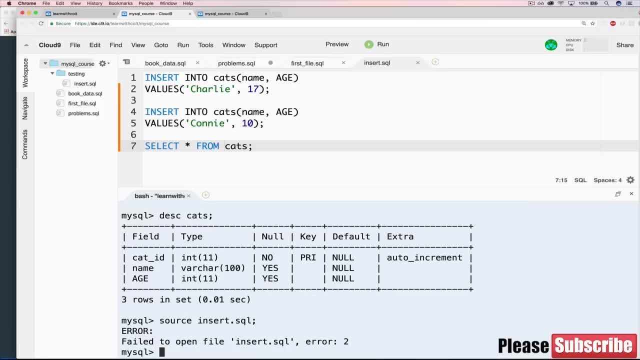 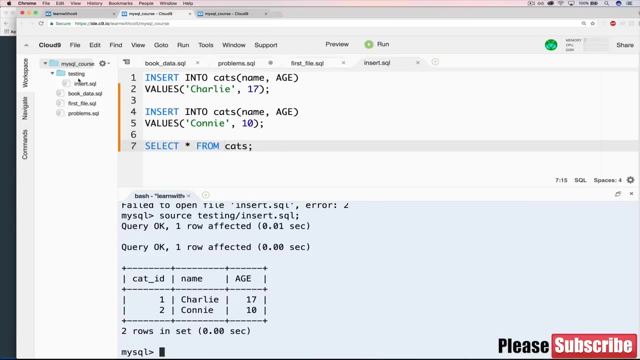 If we did that source insertsql, It tells us it can't find that file. So what we need to do is do a source testing slash insertsql And there we go. So that's important that you have to access the correct path. 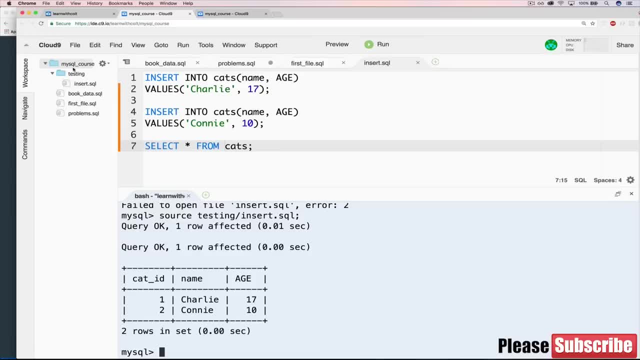 You have to refer to this file by its full path to get there. So if you're in this folder, all that we can access are these. But if we drill to this folder, then we have access And obviously you could extrapolate that to as many layers as you need. 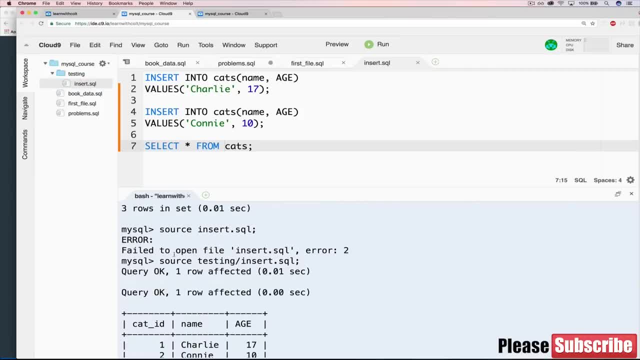 So now let's make sure it worked. You can see after it worked. we had query okay, one row affected. That was our first insert, And then the same thing our second insert, and then our select statement gave us this right here. 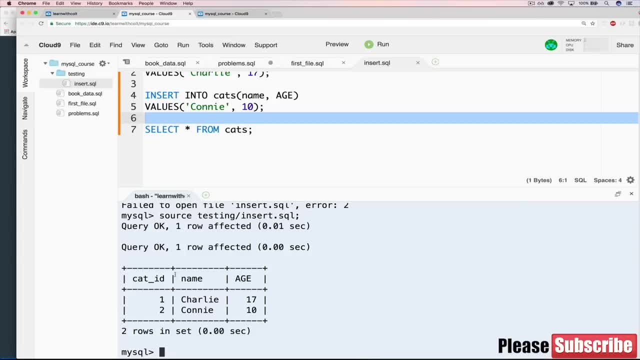 So that's all there is to it. So now that we have access to running code from a file, it's really, really useful. We'll be doing it pretty much nonstop, And the first thing that we're going to do is actually get some new data into our database. 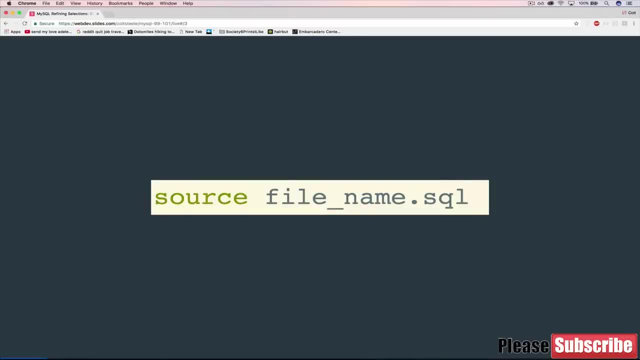 using this in the next video. So now that we've seen how to use source, we're going to take advantage of it to get some sample data going for the next couple of videos and exercises. Cats are kind of boring. They're pretty simple at this point. 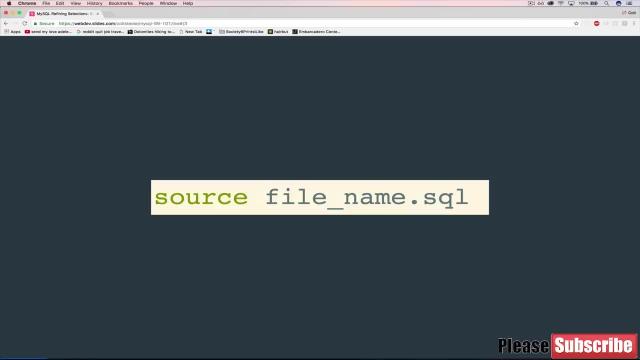 name and age and breed And we need some more complicated data And that's a little something. that's a little more real world. So we're still not working with you know something straight out of a production app, because we haven't seen some of the features. 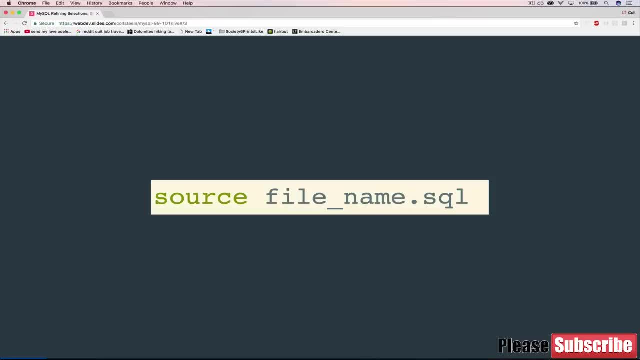 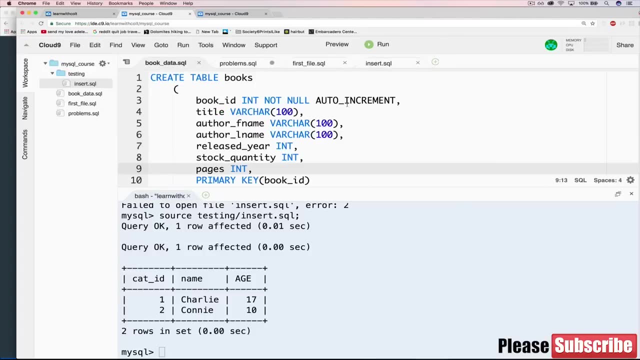 that we need to know for that to work. So it's still kind of simplified data, But what we're working with is books data, So this is what we have. I've given you this file so you can find it in the file section. 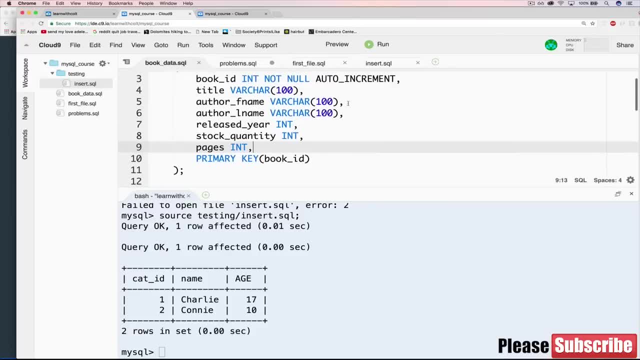 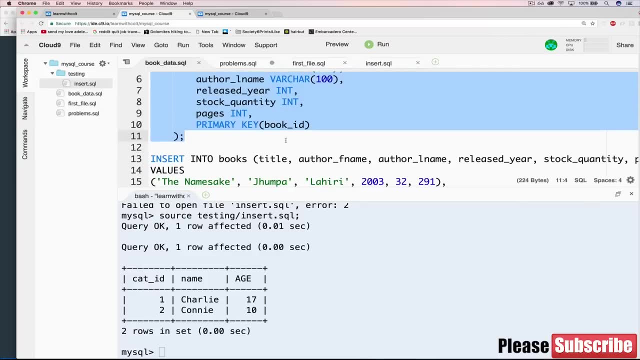 or the downloadable section of this video. Basically, there's two parts. We're creating a books table, And I'll go over that in just a second, And then, after that table is created, there's a bunch of values that I'd like for you to insert. 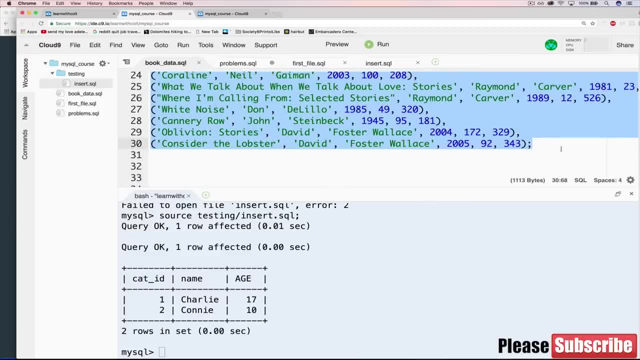 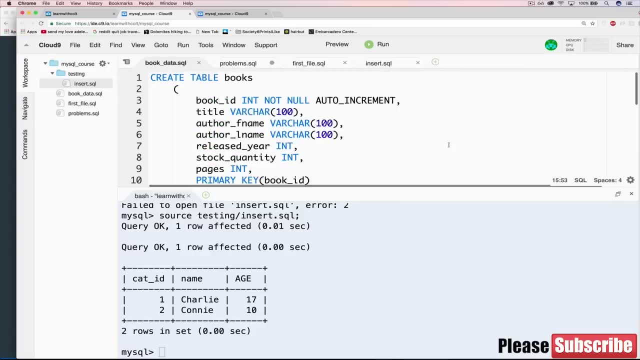 And I didn't want you to have to type these all at once, but I want us to all have the same data so we can be on the same page when we run exercises. So all of this data is actually real data. It's about books from Amazon. 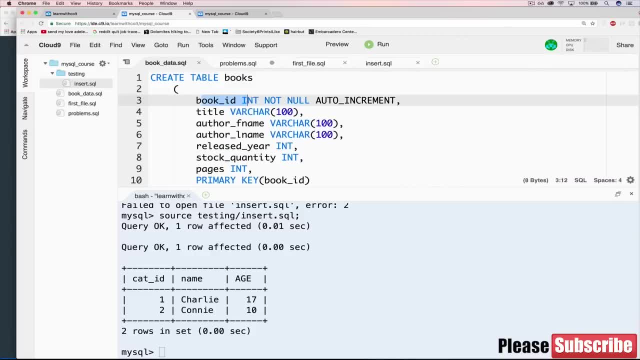 And basically it has. every book has a book ID, So that should not be new. There's a title, It's a varchar. Then we have an author first name and an author last name. So if we look at one, here's the namesake. 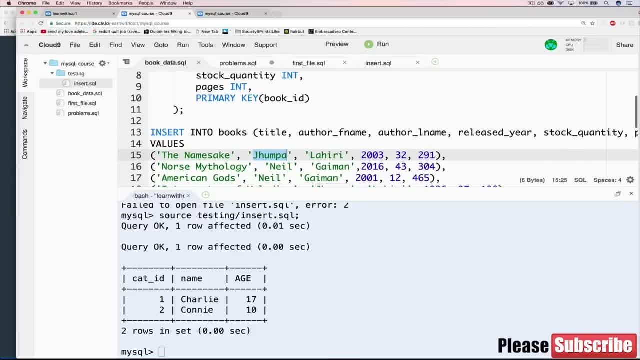 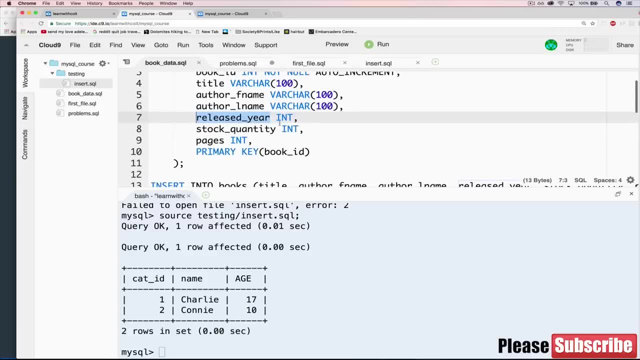 That's a title. The author first name is Jhumpa And her last name is Lahiri. Then we have the released year. So what year was it released in? And this is an example where we're using kind of the. 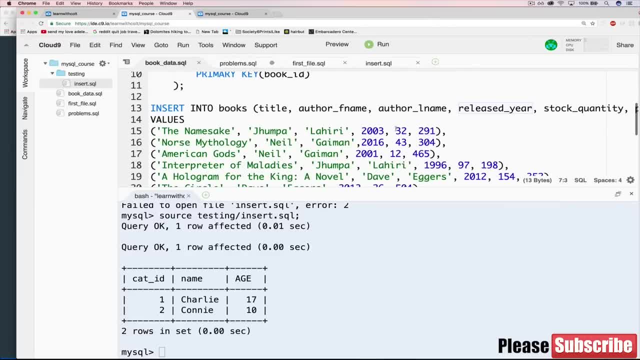 I don't want to say dumbed down, but simplified version of data, Because typically you would probably store a date, an actual date, not just a number like 2003.. So we'll see how to do that once we talk about dates. 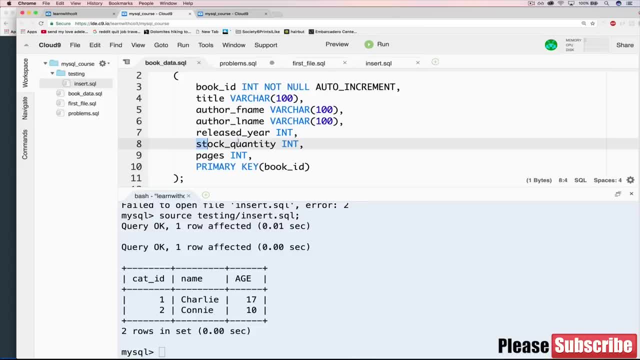 But for now we just have 2003.. And then the next thing is stock quantity, And this is just an arbitrary number I picked. The idea here is that we have a fictional bookshop and we're keeping track of all the books and how many we have in stock. 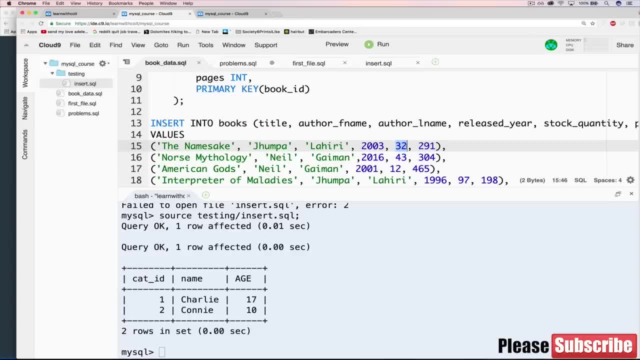 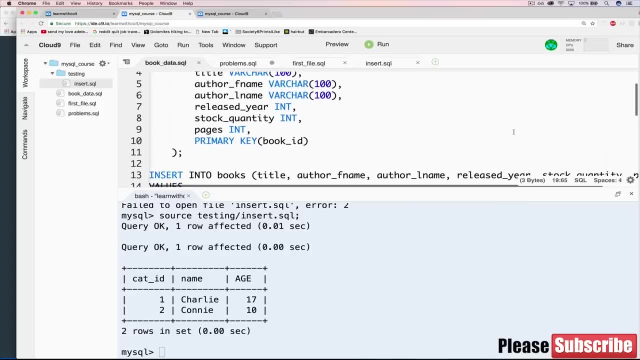 So for the namesake, we have 32 copies in stock. For a hologram for the king, we have 154 copies in stock. Then the final thing is the pages. How many pages are in that book? So you can see some books are really long. 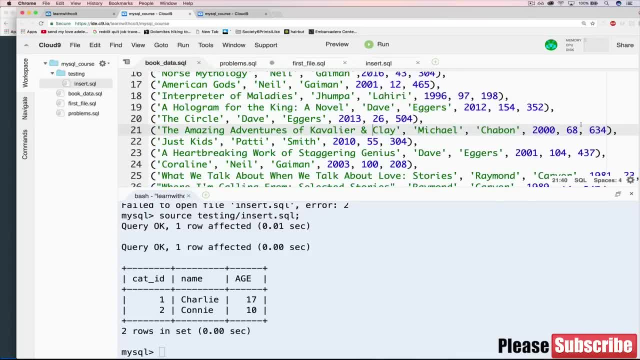 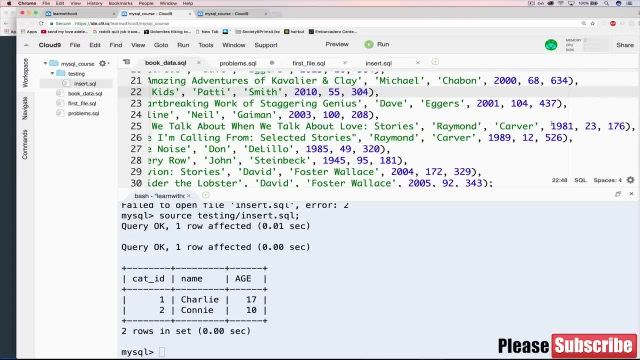 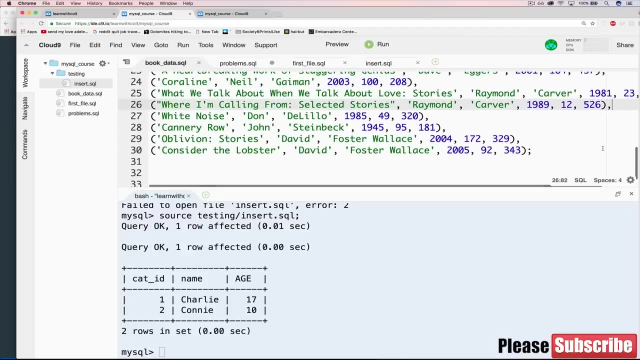 like The Amazing Adventures of Cavalier and Clay, has 634 pages And some are much shorter, like What We Talk About When We Talk About Love by Raymond Carver- Really good short stories if you like short stories- 176 pages. So a note about these books. 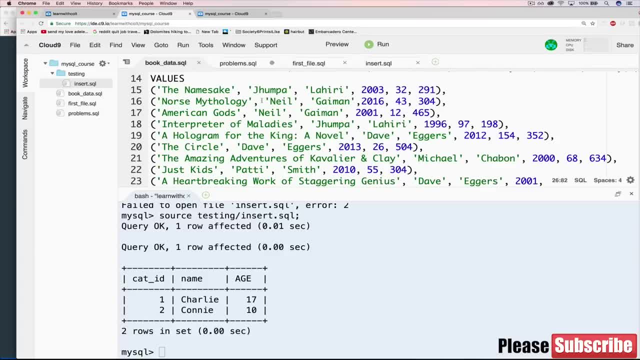 I started off by just picking off the bestsellers on Amazon as of writing today, So I think that's where this one Norse Mythology by Neil Gaiman came from, But I then just decided to create a variety of years and page numbers. 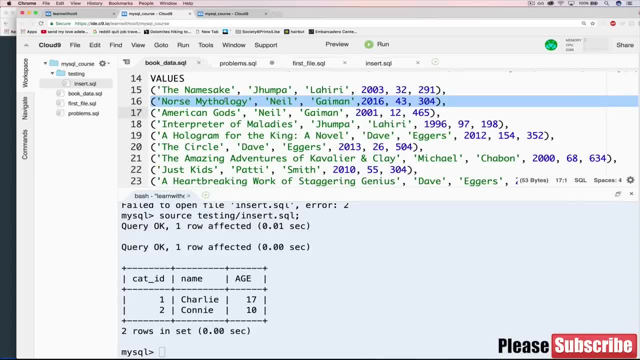 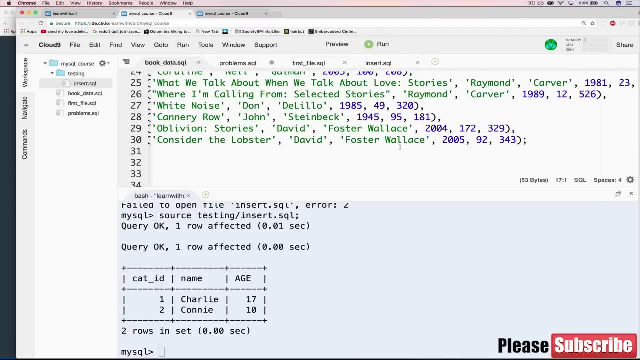 some of my favorite authors. It's a whole mix of things, So it is real world in a sense, but it's also sort of I planned certain things to work certain ways. So we have some really long titles and some short titles. 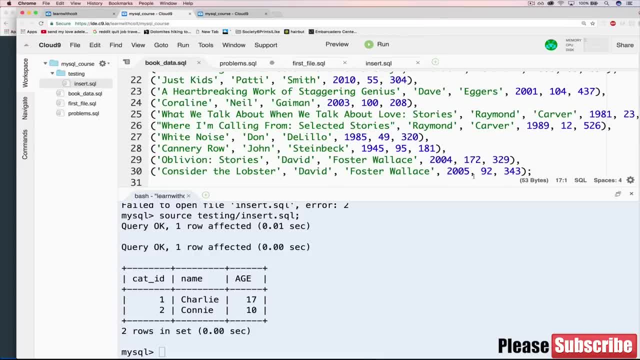 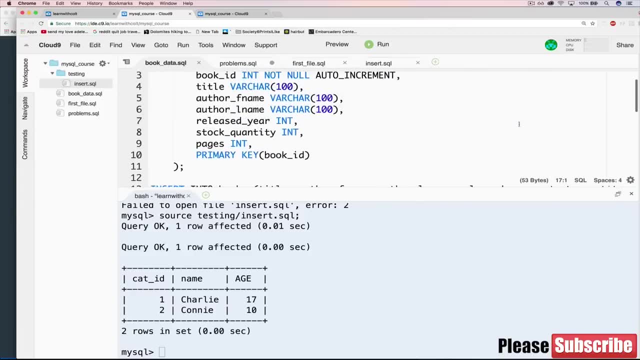 We have some really long books and short books. We have some books from the 2000s and some from the 1900s, and so on. Basically, I wanted a variety of things that we could practice with, So go ahead, create a file in Cloud9. 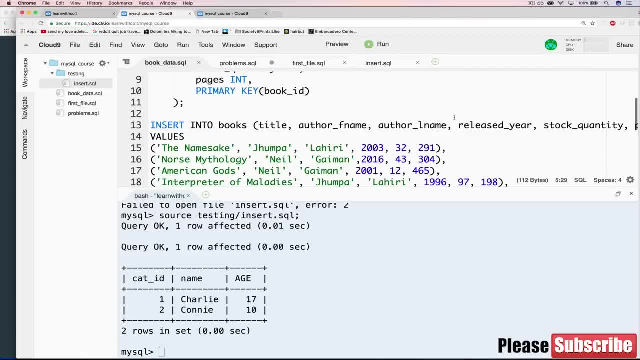 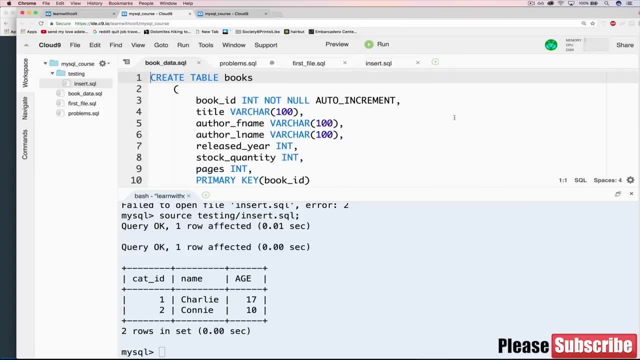 and put all of this in there. Now, if you want to type it, go ahead, But I would recommend that you don't, just so that you don't accidentally mess something up. We want our data to be consistent, So go ahead. copy it. make a new file. 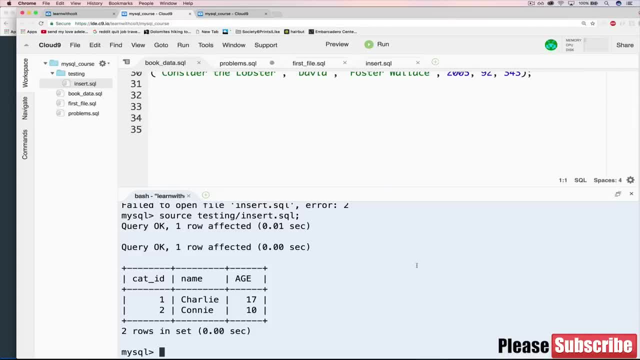 And then we need to execute that file And I want to make a new database Right now. if we do select database, we're working with CatApp. I want to create database and we'll call it bookshop And then use bookshop. 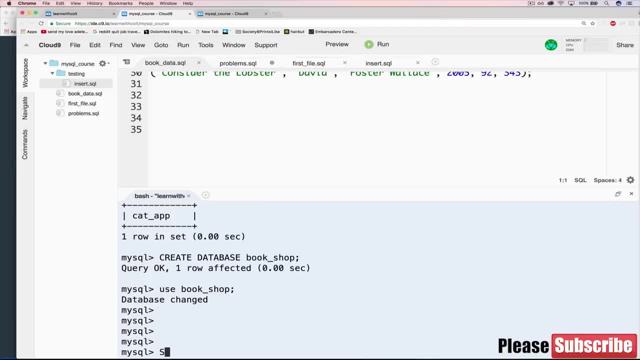 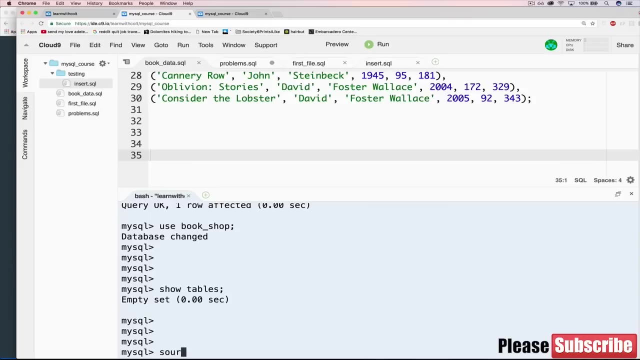 And we should have a blank slate. If we do show tables, there should be nothing here, Perfect. So what you want to do is make sure this file has been saved, And then we just execute it. So it's pretty straightforward. Source. 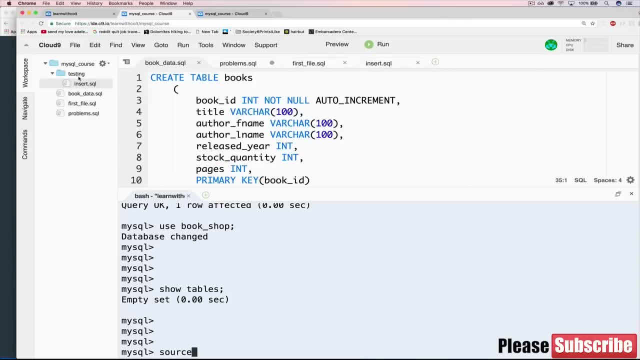 And then you'll need to make sure you either are referencing the correct path. So in my case, I'm running my CLI in my root directory, So all I have to do is bookdatasql- Whatever you called it- you'll need to refer to. 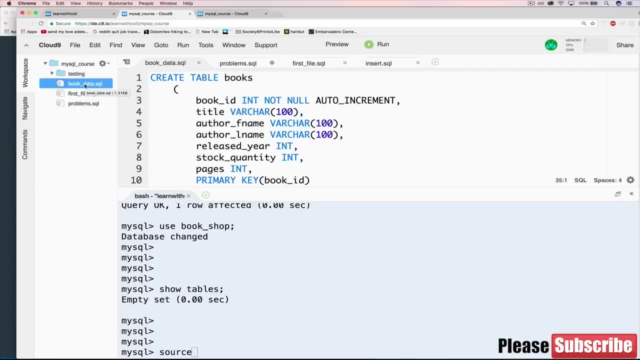 I recommend just putting it in the main directory for now, But you could have a separate folder if you wanted to, And you just need to refer to it correctly. Anyways, source: bookdatasql. And here we go, All right, First thing, 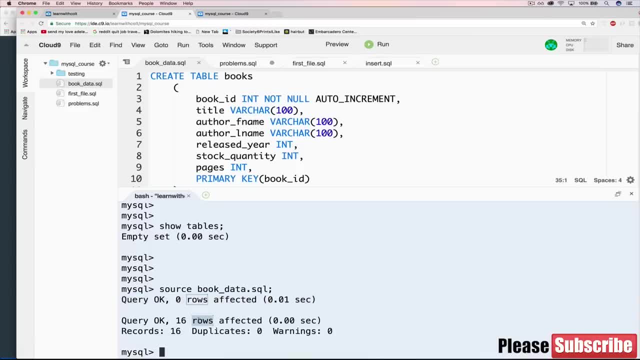 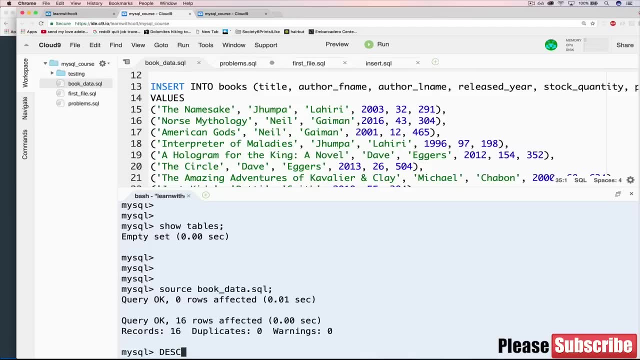 We get this message And that tells us the create table worked. And then we get 16 rows affected And that tells us the insert statement worked. So let's just verify, Let's do describe books. Here we go. Here's all that we created in that table. 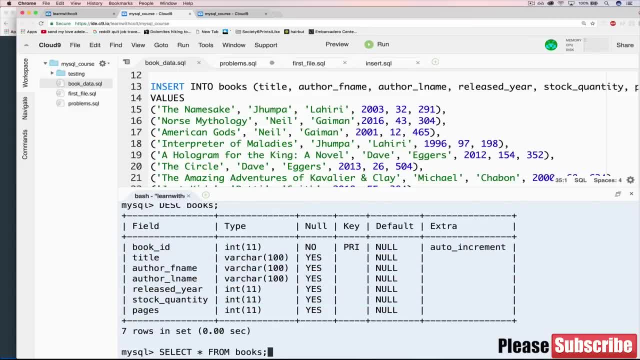 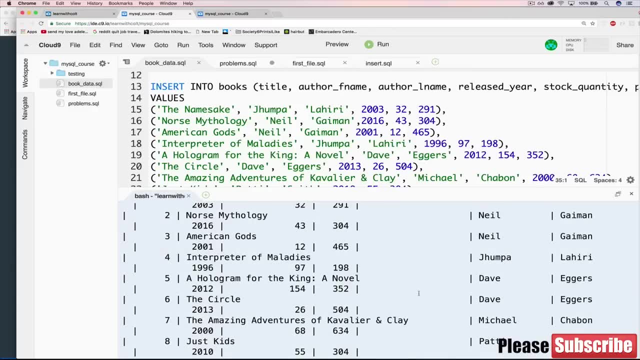 And let's just do a simple select star from books. As you can see, it's pretty messy And that's deliberate. That's deliberate. We're going to work on ways We're going to see ways of refining this and making things shorter, collapsing data and so on. 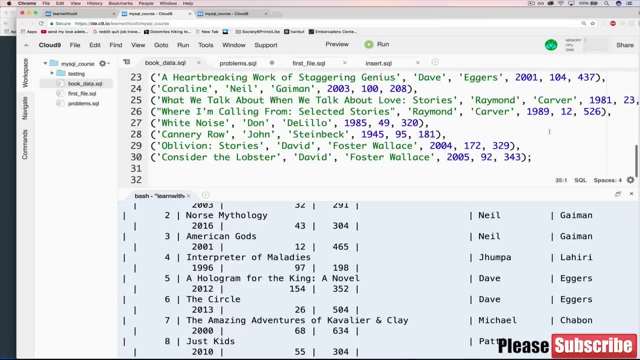 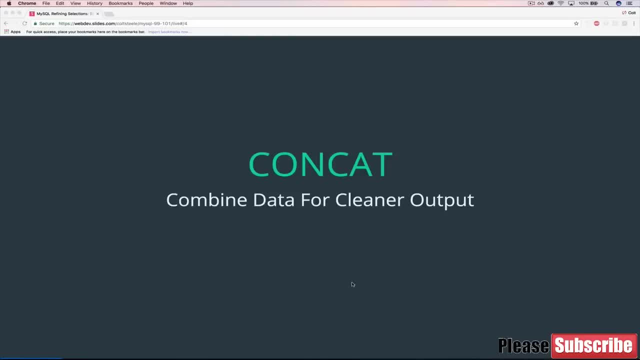 So that's all we're doing in this video: Just getting set up. Now that we have it in there in our database, we'll be able to work with it and be on the same page. Awesome, All right, So we have that out of the way. 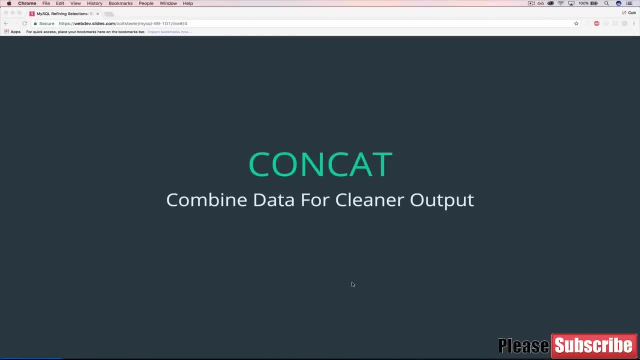 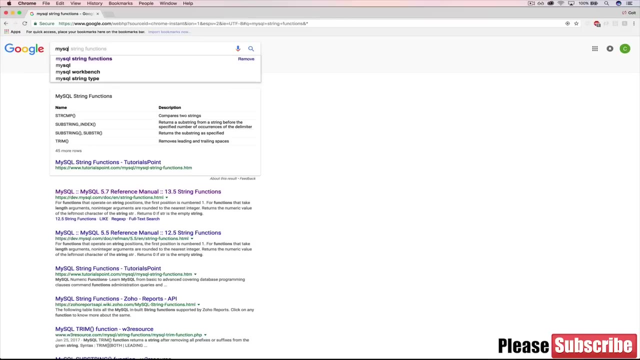 We've seen how to run files using the source command, And then we actually did that with the sample data that I gave you. Now we actually dive into the meat of this section, which is all about string functions, And the first thing I want to show you is that if you go to Google and we type in MySQL string functions- 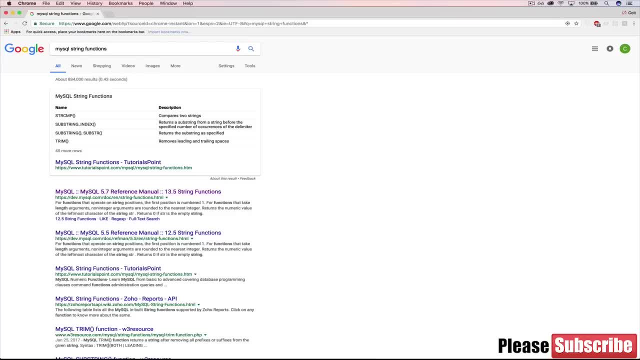 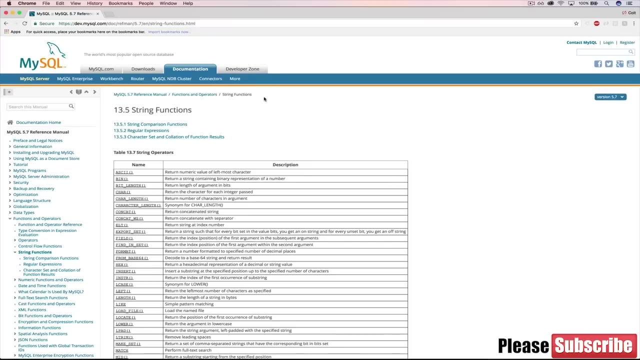 Whoops, String functions. Excuse that. And we hit enter here. You can see I've already clicked on this link: the MySQL reference manual- string functions. I have to say I'm not a huge fan of the documentation of MySQL. For one thing, I think it's kind of ugly and looks dated. 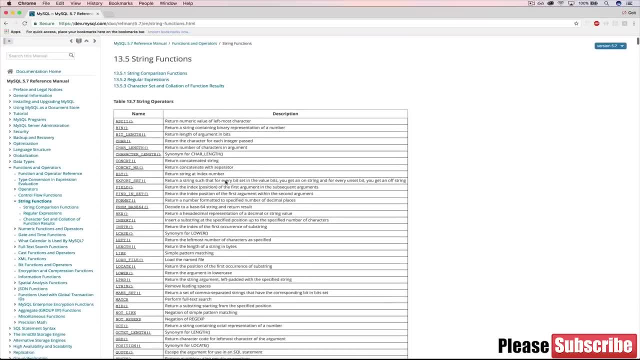 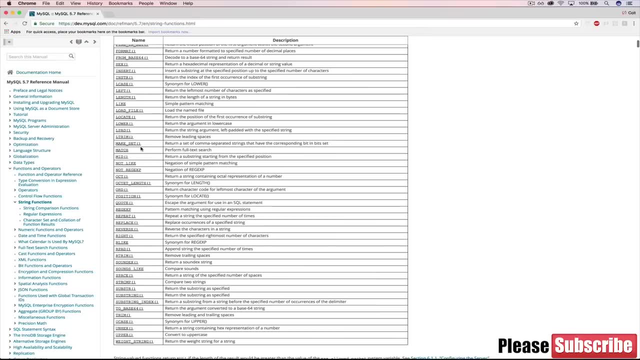 But it does have all of the information you need. I just don't really like how it's presented, But if you look at this giant list here, these are all string functions that we can use, And a lot of them are very, very specific. 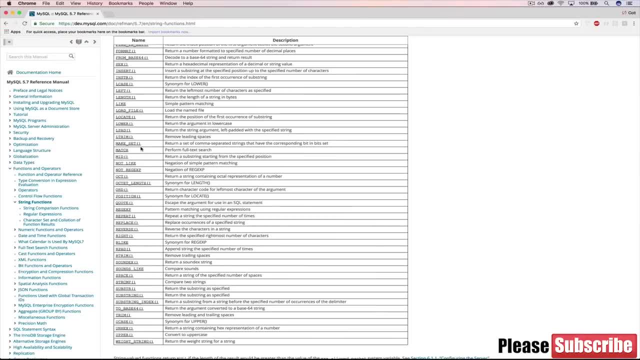 I'm going to show you some of the more well, first of all the useful ones, and then a couple of just fun ones, And that we'll be able to combine together for some good exercises. But we're not going to take a look at most of these. 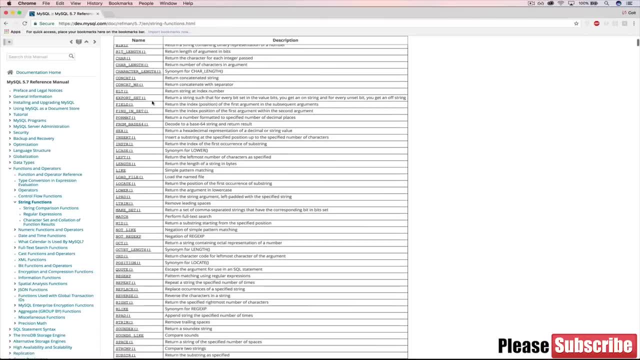 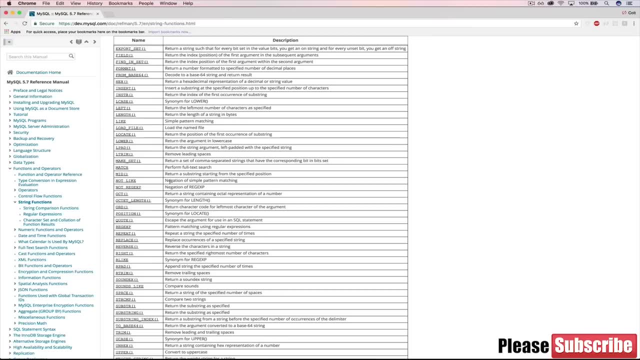 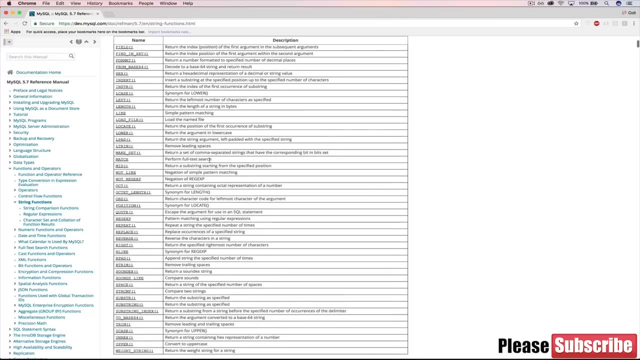 Most people don't even know that these are here. I'd say That's a generalization, But in my experience working with MySQL and people who work with MySQL, you use maybe five of these on a regular basis And then occasionally you might need to do something like: hey, is there a way of doing X? 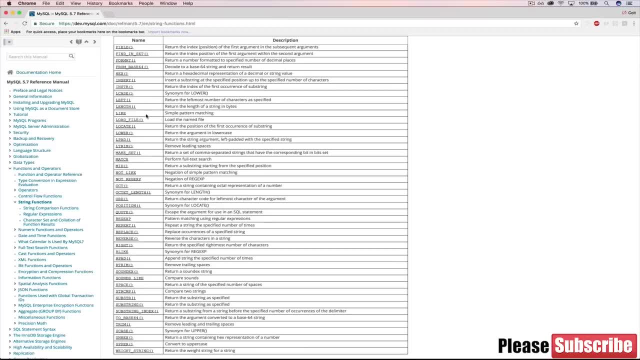 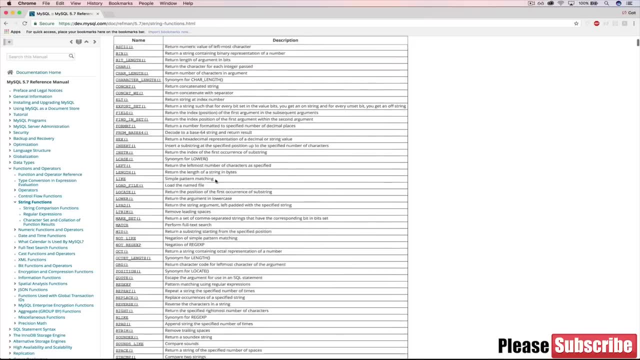 Let me go check on the documentation And, oh look, there is a way of doing that, Perfect. Or oh, no, there's not a way, Great. What am I going to do next? So I just want to show you that this is here. 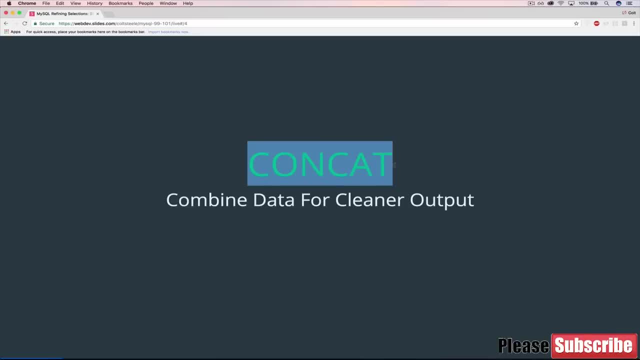 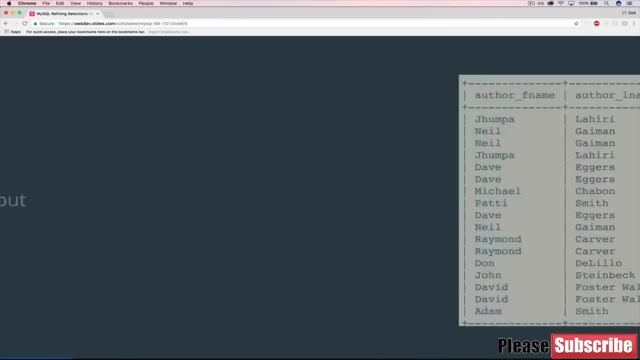 And the first one that we're actually going to take a look at Is called concat. So what it will do is combine pieces of data, Combine strings. So here's an example using this book data. Remember that we have author first name and author last name. 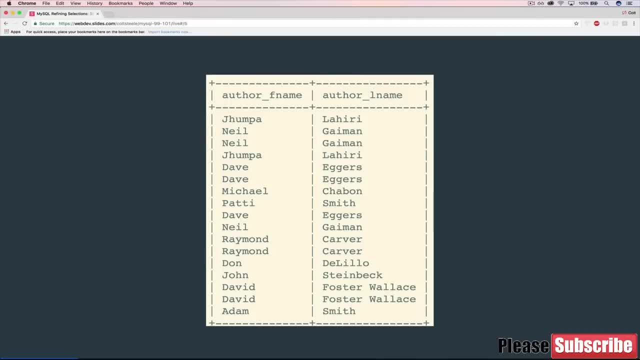 And there are valid reasons for separating that data. Sometimes, I mean, you might want to sort books by last name, And sometimes you may only want the last name. in certain contexts You might not want the first name. It's not a great example. 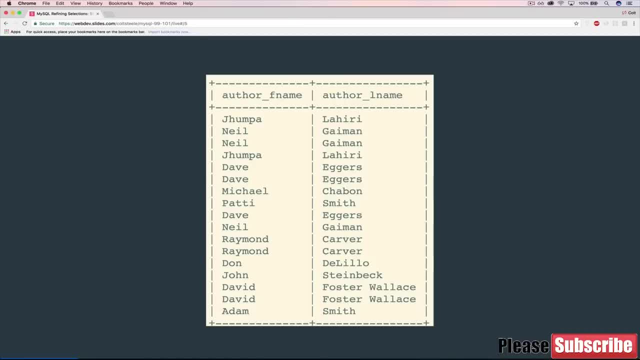 But there are reasons that you would separate this out. Just like when you're filling out a form online, You're signing up for a site. They usually don't just ask you for your full name. They ask you for a first and last name. 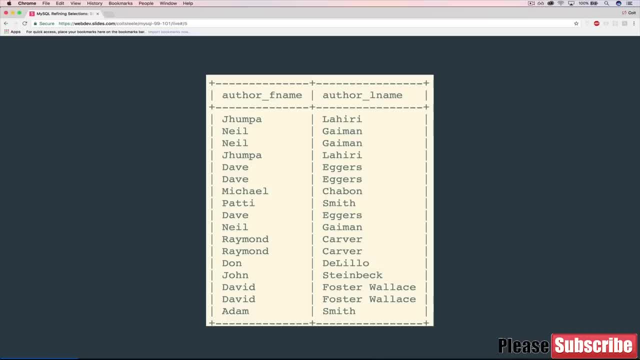 But then if they have those pieces of information, it's pretty easy to combine them. So that's what we're going to see now. How do we combine these two and get something that says Jhumpa Lahiri or Neil Gaiman? 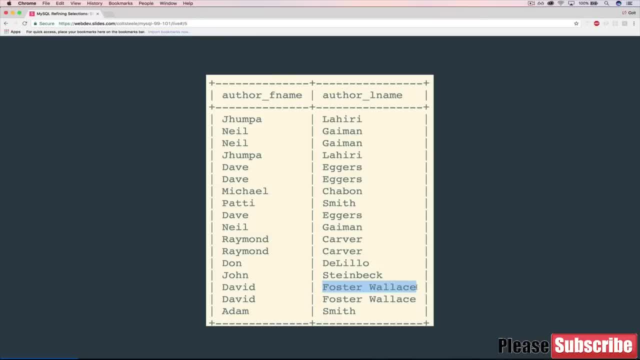 Or in this case, Foster Wallace as the last name, Which I'm actually not sure if that qualifies as a last name exactly. But David Foster Wallace, How do we combine that? How do we get that? And the answer is: we use concat. 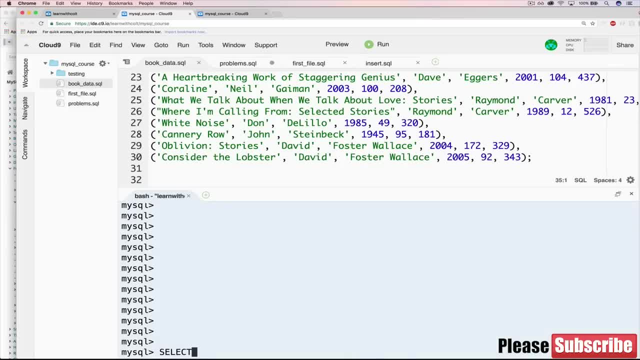 So let me just first show you what we have right now. We'll do a select author fname, author lname from books, And that's what we get here, Just what I had printed out in the slides. So what we want again is to combine them. 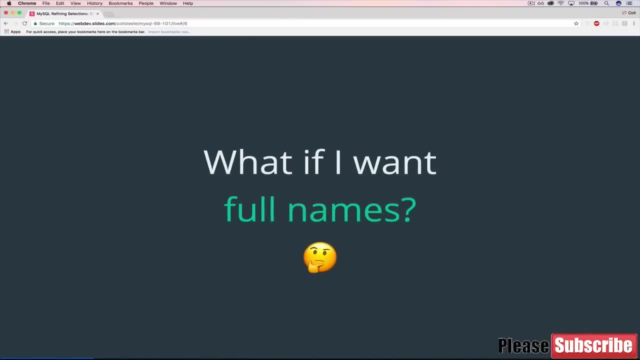 But we'll take some baby steps And yep, here's a slide. I totally got ahead of myself. What if I want full names? So concat. The way that concat works is that we pass in multiple arguments or pieces of data. 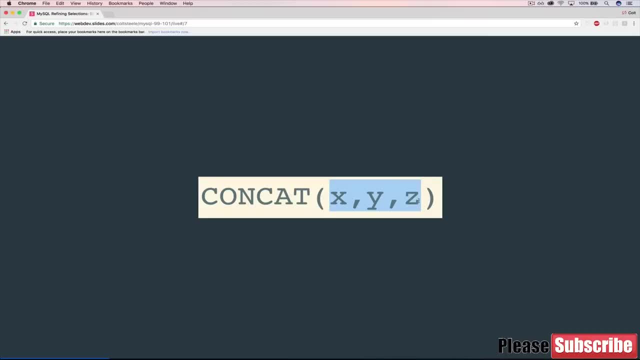 And it will combine them. So, whatever we give it In this case, I mean, if you had columns named x, y and z, this would work, But it's really just supposed to be an example. More specifically, what you can do are things like this: 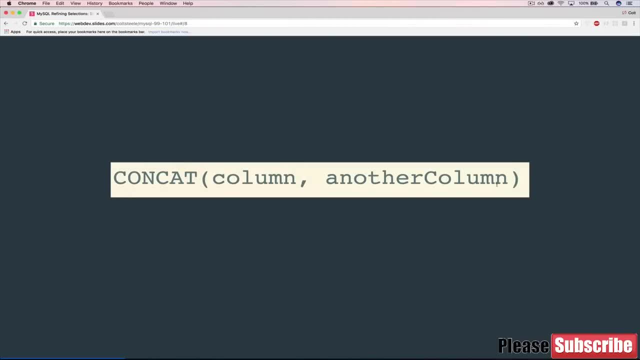 Concat a column name with another column. So that's what we'll work on. We're going to do author fname and author lname and combine them together, And if we do this right here- So concat author fname and author lname- What it will actually do is just slam them together. 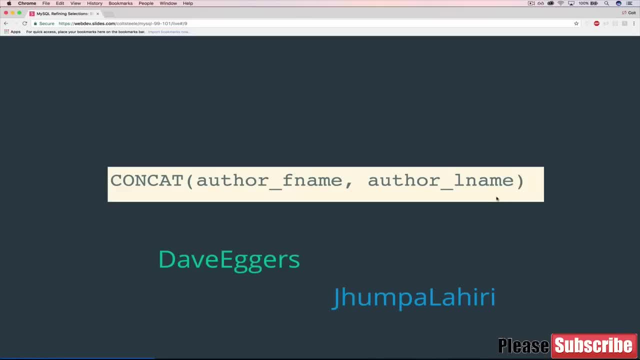 Put them exactly together, Concatenate them, So there's no space in between. So we get Dave Eggers, Jhumpa Lahiri, So there's no. you know, that's not exactly what we want. Maybe we want a comma. 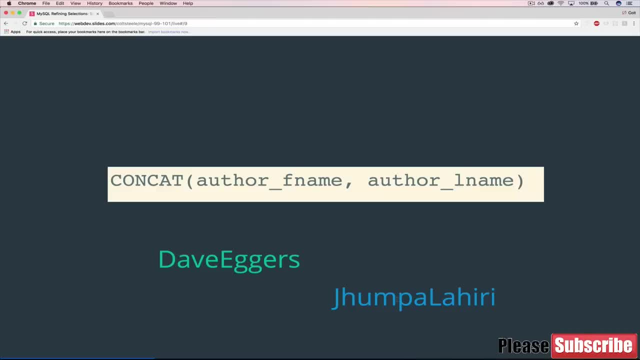 Maybe we want last name, comma first name, Or maybe we want first name, space last name. So there's a way of doing that. When we concat we can pass in a column name And then some other text And then another column name. 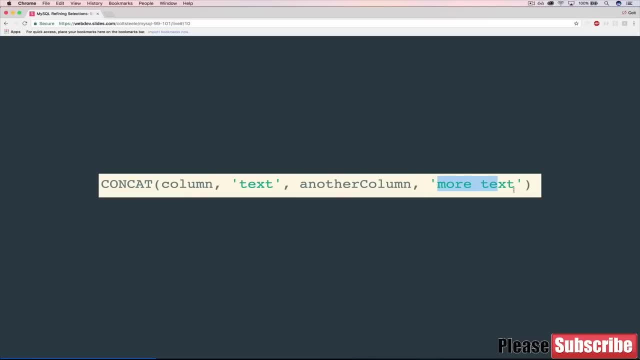 And if we wanted more text, And we can keep going on and on and on And it will concatenate everything. So to add a space, it's pretty simple: Author- first name comma And then a space comma. author lname. 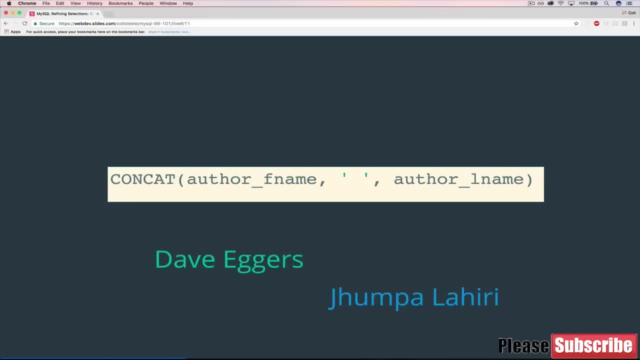 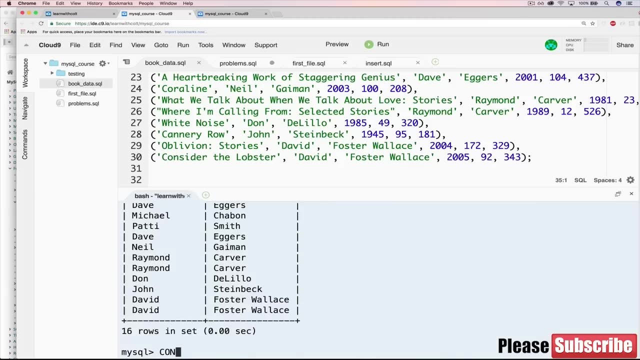 And that will give us Dave Eggers and Jhumpa Lahiri. So now that I've shown you in the slides, let's take a look. And the first thing I'll show is that often people expect they can just come in here and just type concat. 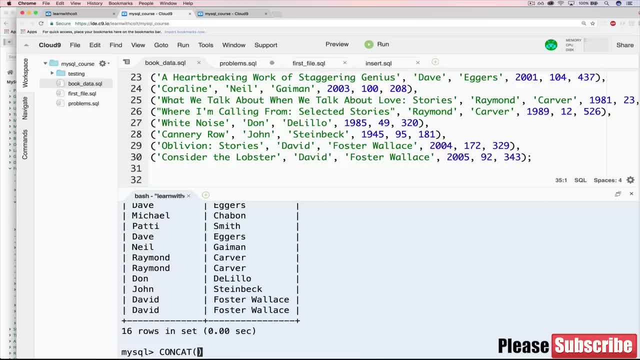 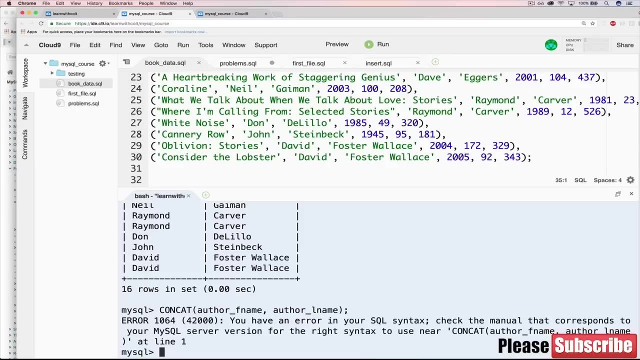 But if I just do concat well, author fname, comma. author lname, There's a problem. Hopefully you can identify what the problem is. If I hit enter, this is not valid syntax. First of all, it doesn't know what table. 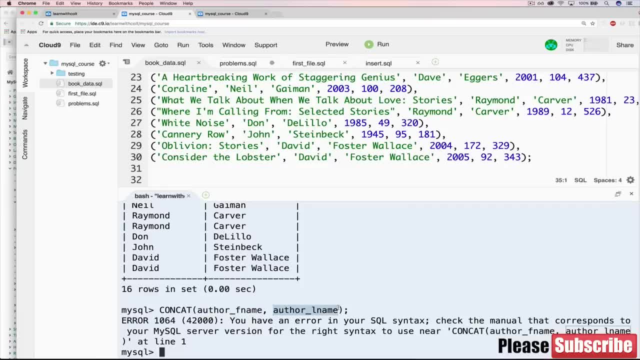 What if we have multiple tables? Where's author fname coming from and author lname? And second of all, we have to select. So we can't just run these willy-nilly, We can't just run them on their own, We need to run them as a select. 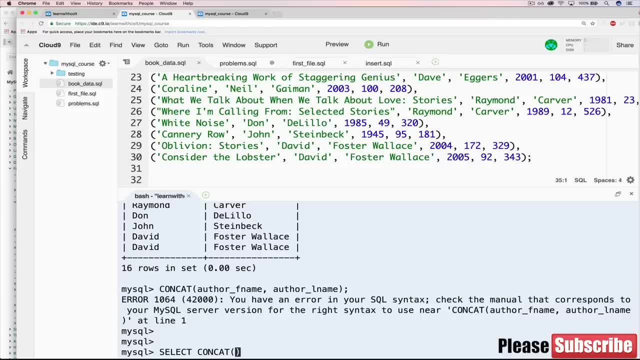 So select concat. And then in here I'm actually going to start with something simple. I'm not going to use columns, I'm going to use text. So I'll just put something like: hello comma world. So this is very trivial. 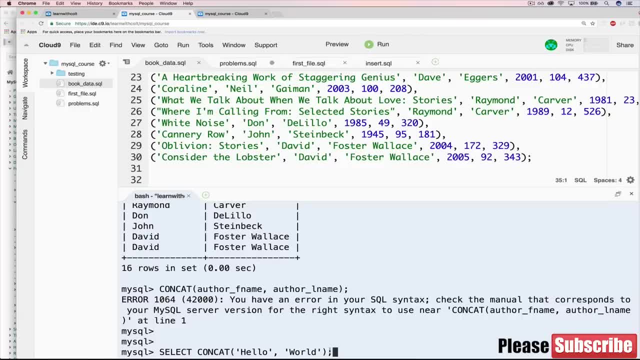 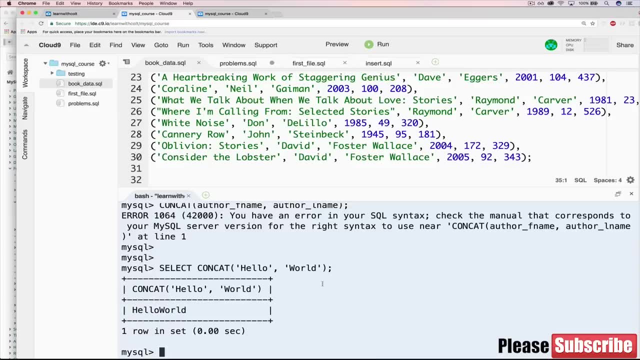 But if I just do this select concat, hello world And I hit enter, You can see it does it for me And it just gives me hello world combined to these two things. So I could do the same thing and add a space. 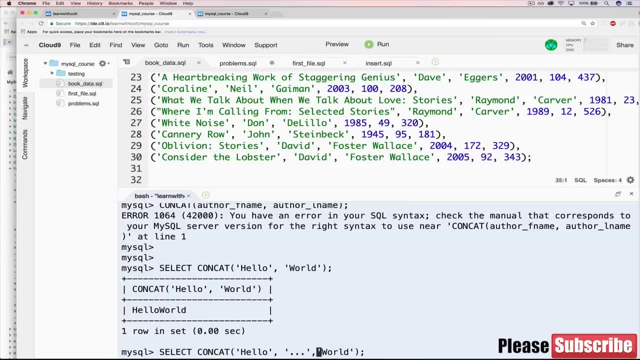 And rather than a space, let's do dots so it's easier to see, And we need a comma. A lot of punctuation going on. Select concat, hello comma, dot, dot, dot, comma, world. It just shoves them all together. 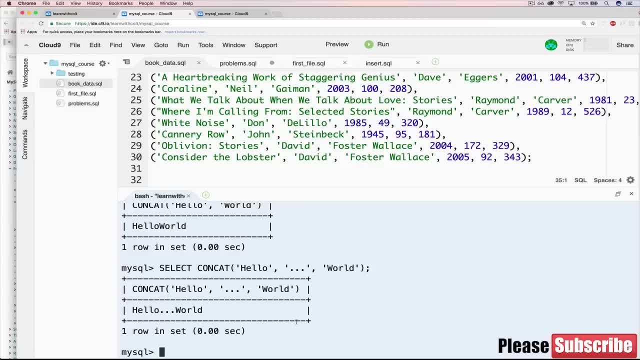 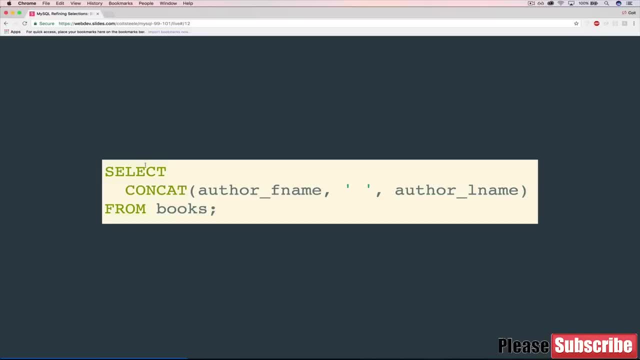 And we get hello dot, dot dot world. So that's how we can do it with just text, which you probably won't be doing. You'll be doing things like this: Select And then concat a column like author: F name. 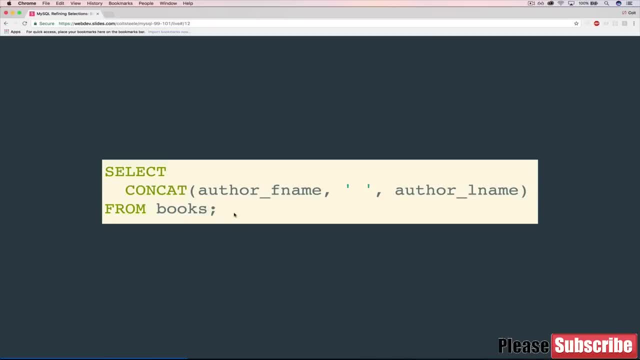 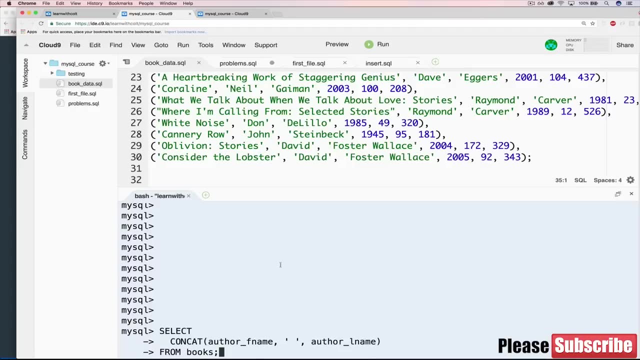 And then a space And then author- L name from books. So let's try it. We can copy it now. Go over here and paste it, Select, And what it will do when we hit enter is just make a new column for us. 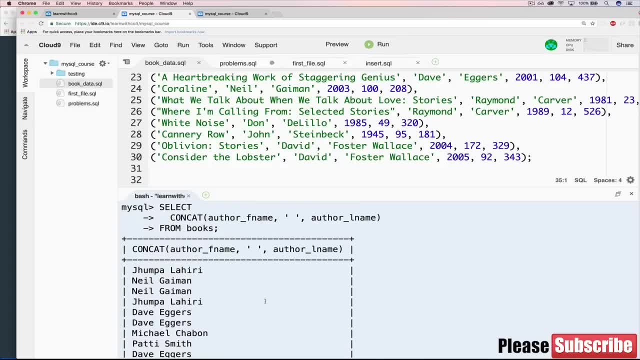 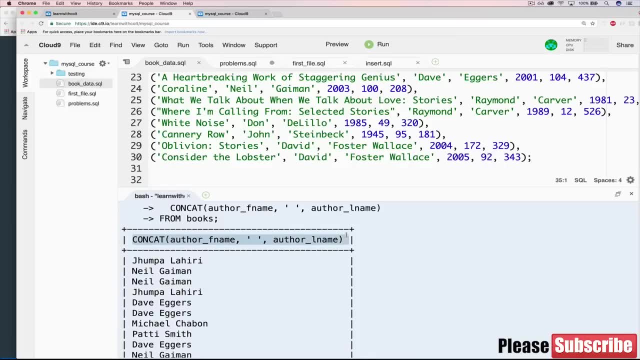 Or in our results. It doesn't change our initial data. just to be clear. Our data looks the same in the database. This is purely about printing it out. But we have this new thing up here with this horrible title: Concat. author F name. comma space comma. author L name. 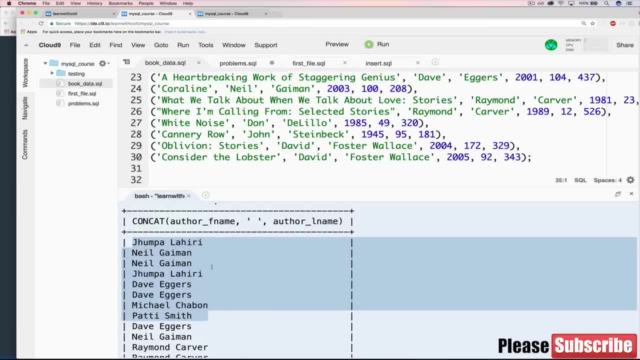 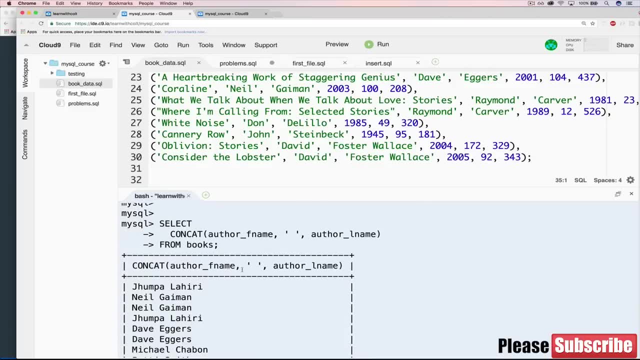 But then in here we have the data that we're looking for. We have Jhumpa Lahiri, We have Patti Smith, Raymond Carver And so on, So that's really useful to combine data like that. Now, if we want to get a little fancier, let's rename it. 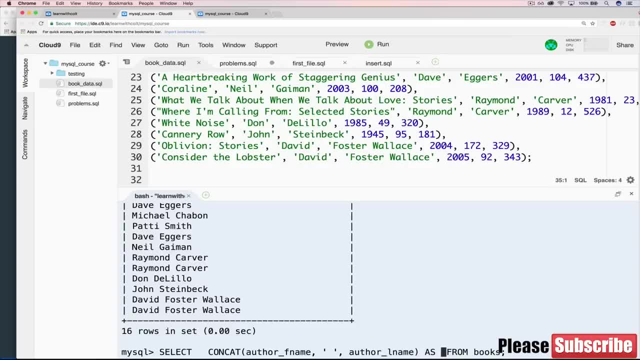 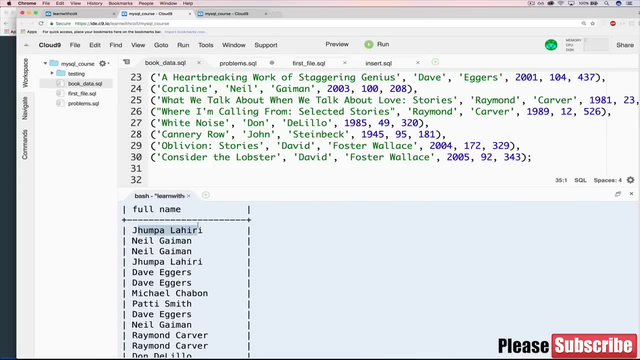 So let's give it an as, And we'll just say as full name, Just like that. And now I get full name up here: Jhumpa Lahiri, Neil Gaiman and so on. So that's concat. 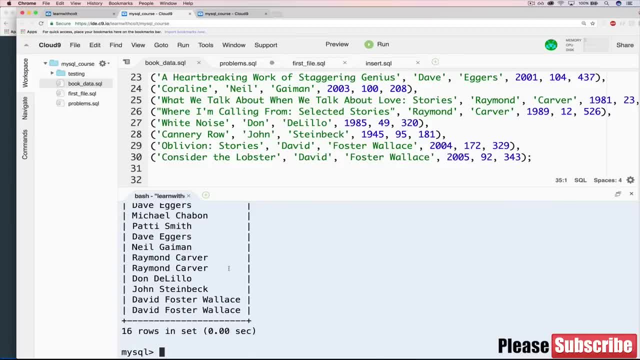 I'll show you a couple more examples, Just to show you how these string functions work. You don't have to just do one at a time. We could do something like this: Select, And we'll do author first name just on its own. 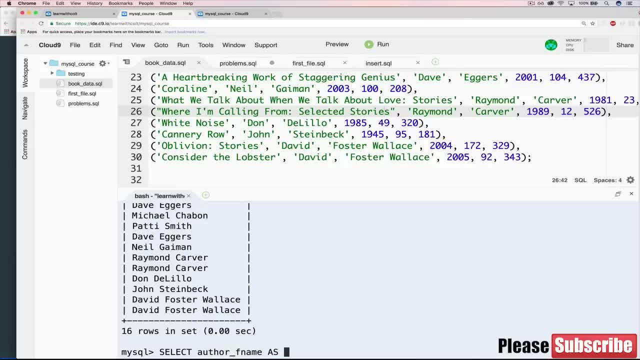 Author F name. Author F name as first name. Let's just do first actually As first comma author L name as last, And then we'll have a concat author. And let's do it on a new line, just because it gets a little messy here. 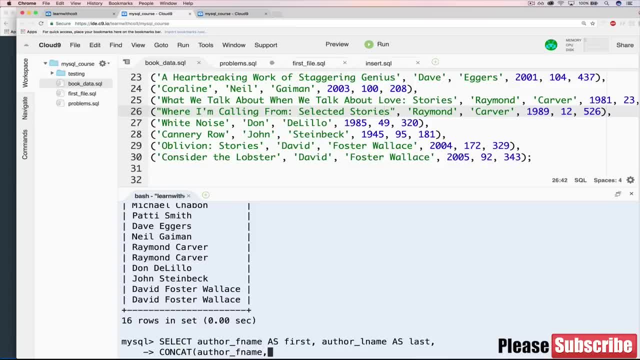 Concat. author F name. This is what we've already seen, With a space comma. author L name as, And we'll call it full. So we'll have three different things printed out: The first name under the title first. Author L name as last. 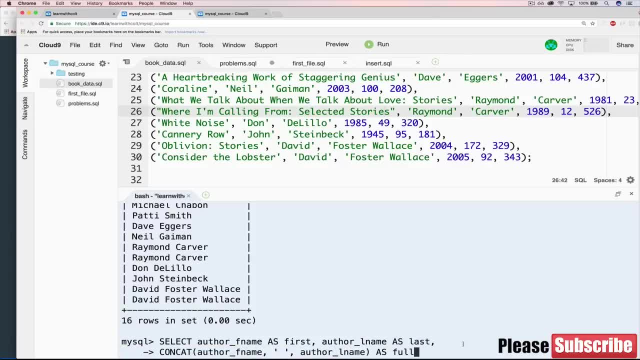 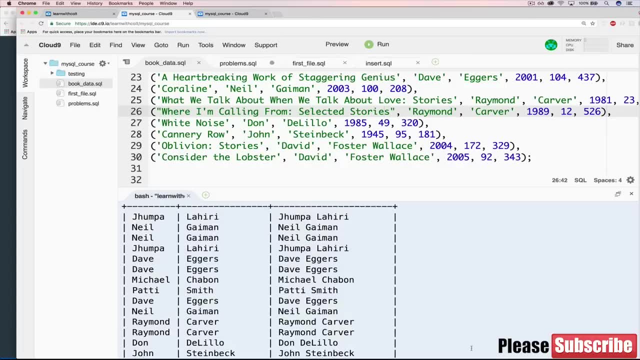 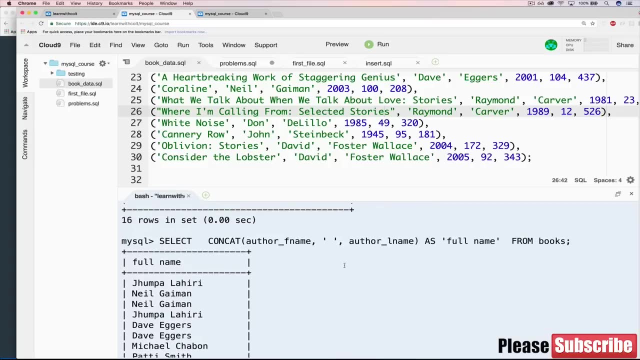 And then the full name combined, using concat as full. So then we need to say from where? From books. And now I hit enter And I get this pretty little table First, last and full. So what I want to show is that you don't have to use it in isolation. 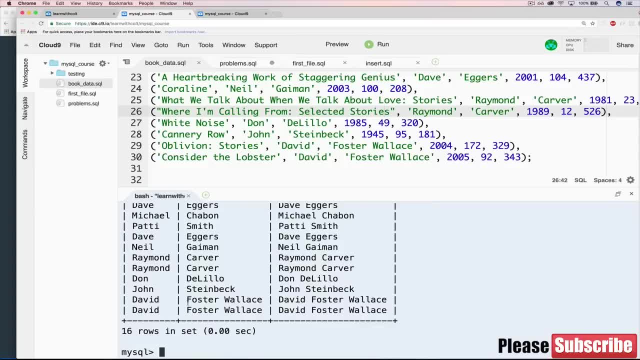 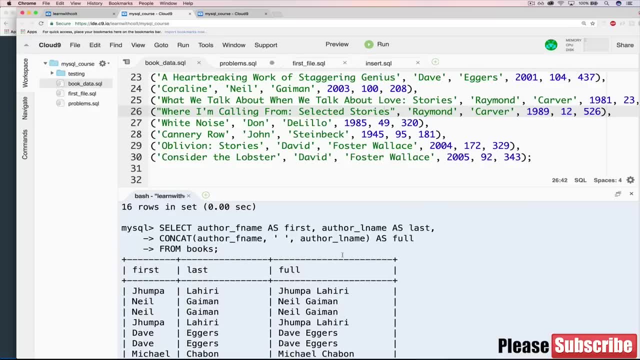 You can combine it with other things And we'll see this as we go. We're not going to just use concat And you don't have to just use one concat per select. You could have multiple if we wanted to. You know, I could have full name. 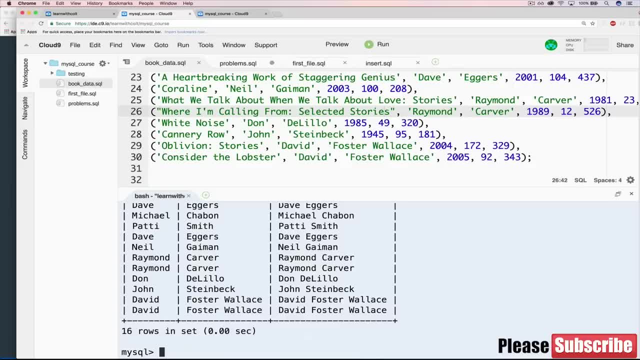 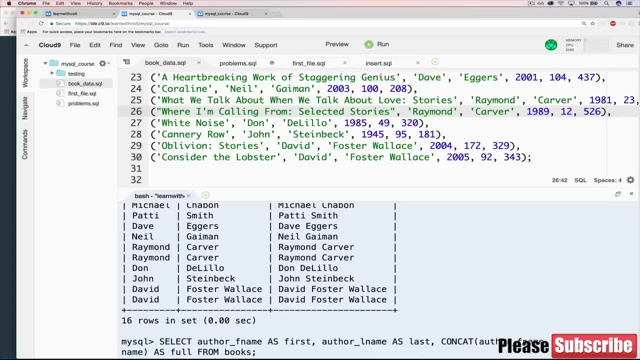 And then I could have full names comma separated instead, And if I wanted to do that, you can probably figure this out. But rather than just having a space there, I'll just put a comma. And now I get Jhumpa, comma Lahiri. 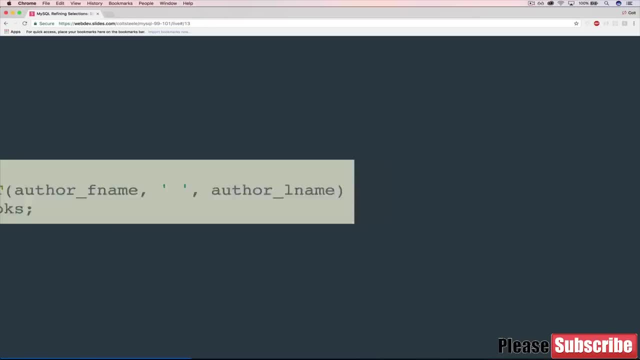 All right. So one more thing about concat is that there's something called concat WS, Which stands for concat with separator. So there might be times where you're concatenating multiple fields, Multiple things together with the same symbol or piece of data stuck in between them. 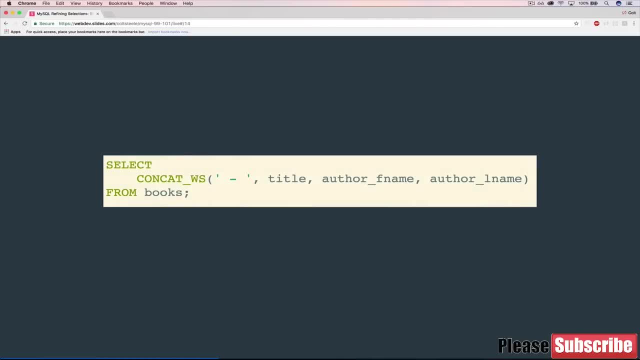 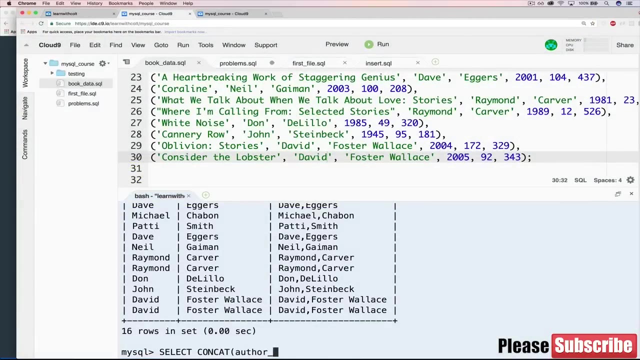 So there's a shortcut for that. So if I wanted to have title dash author, F name, dash author, last name, Let's not debate why, But if I wanted to, I could do something like this: Select concat And we have author. 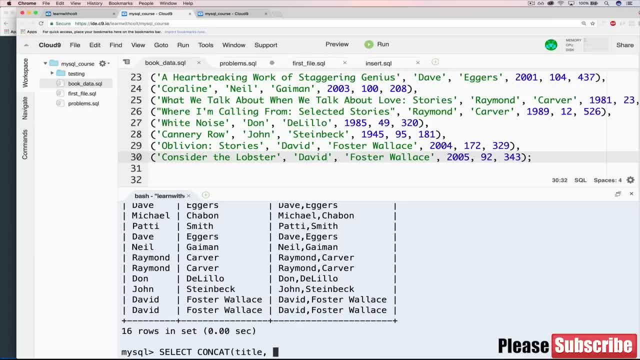 Or actually we started with title Comma And then we wanted a dash, And then author F name comma, And then another dash Comma, author L name, Just like that. So it's kind of a lot of repetitive typing, Especially if we have more items that we're combining. 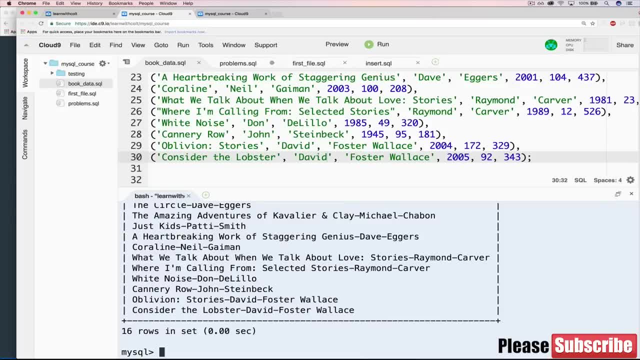 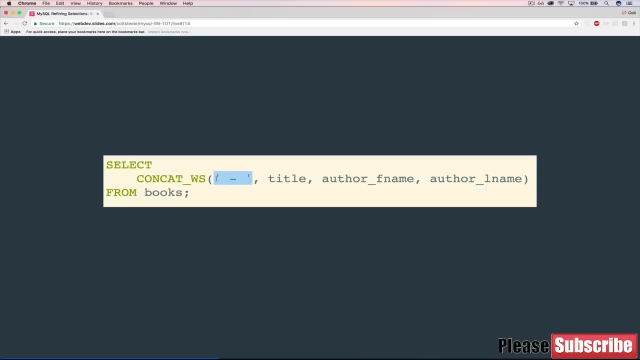 But if I just do this here From books, You see it does what you expect. It puts the title dash first, dash last. But we can use concat WS And it looks like this. So it switches things around a bit. The first thing that we pass in is what we want the separator to be. 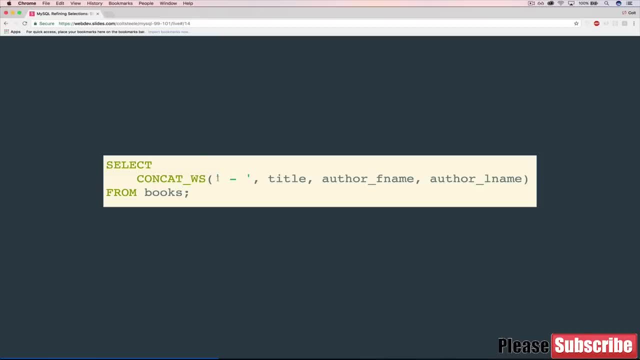 So in this case, a dash with a space on either side, And it will go ahead and then insert that in between every other thing we pass in. So we'll have title: dash author first name, dash author last name. So now, if I paste that in, 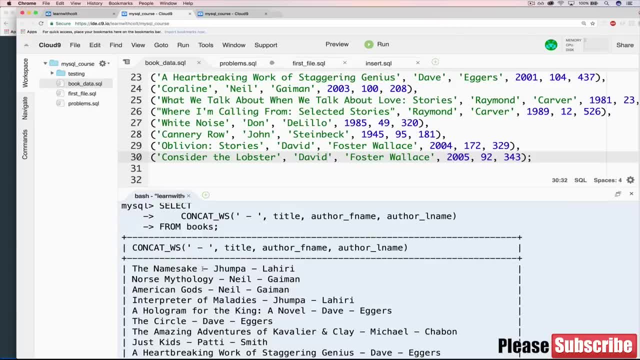 You can see we get the same result, Although I added spaces here, But it's the same idea. It's sandwiched every time, So just worth noting If you ever are in a situation where you're combining lots of data in the same manner. 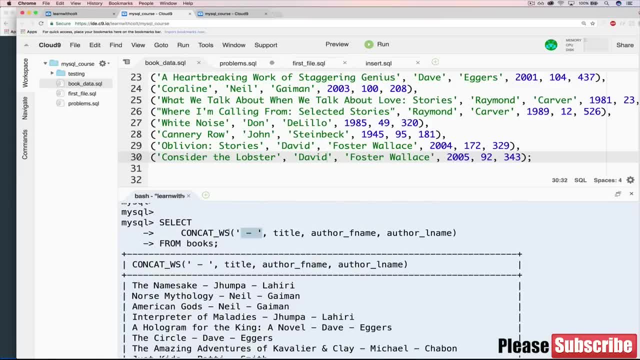 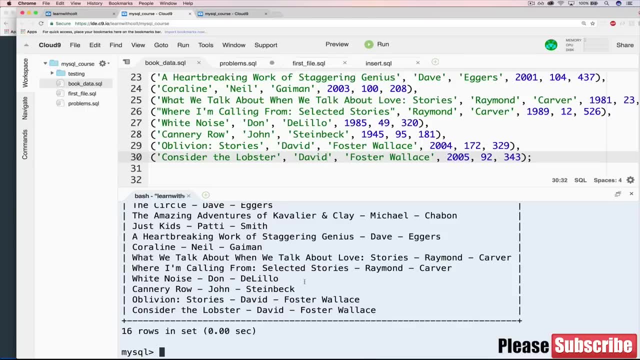 You can use concat WS to save you typing this order Or whatever your symbol is Over and over. So that's our first string function. we saw Concat and concat WS And what they do is concatenate Or shove together, Smash together strings. 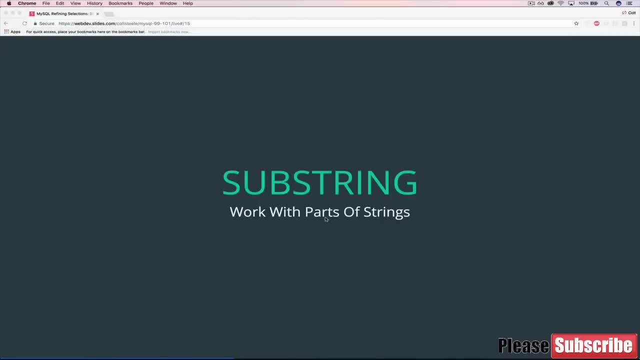 Next up in this onslaught of string functions Is substring. So substring allows us to select individual parts or portions of a string. I only want the first character, I only want the middle ten characters, Or the last character, or so on. So the syntax is similar to concat. 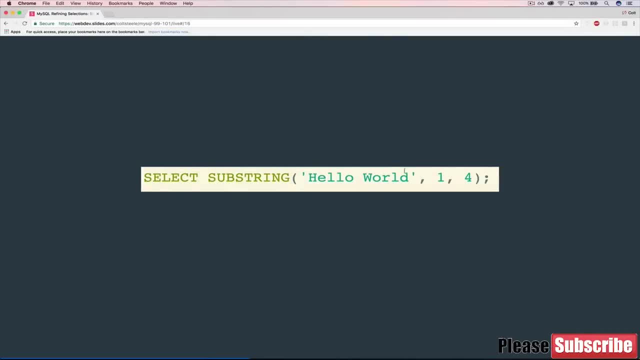 Here's an example. In this case We're not working with columns or tables or anything. We're just working with static data. Hello world. And what this will do: Select. So there's our select again, And then substring, our string function. 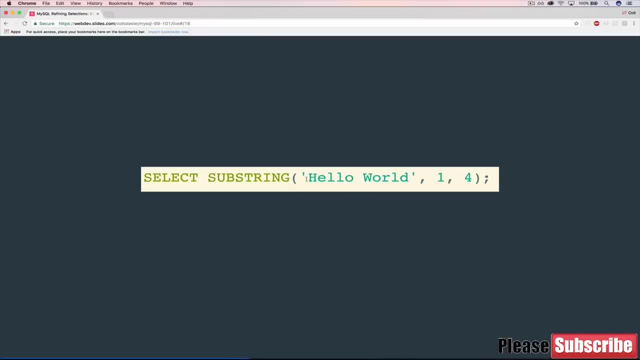 In parentheses. In this example, The first thing we do is tell it: Here's the string we want to work with, So that first thing is hello world. And then what we're going to do Is only print out The substring. 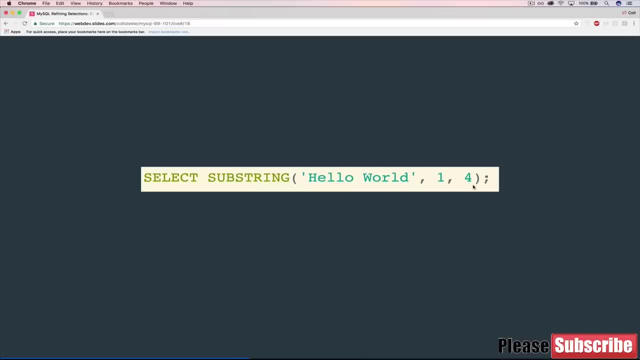 The portion From one to four. So those are indices Referring to characters, And in MySQL They start at one. If you're familiar with other programming languages, They often start at zero. That's not the case here, So H. 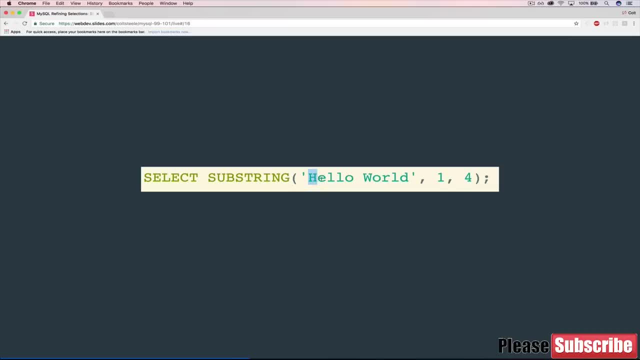 Is one, So we go from one to four. So one, Two, Three, Four, Which gives us Hell. I'm sorry, That is a bad word. Please don't be mad at me. So, Hello world, One to four. 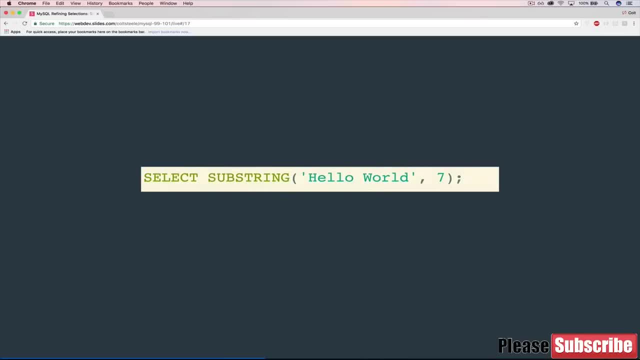 Gives us that, But that's not the only way of using it. Here's another example: Select substring. Hello world, The same starting piece of data, And this time All we give it Is One number, One index: Seven. 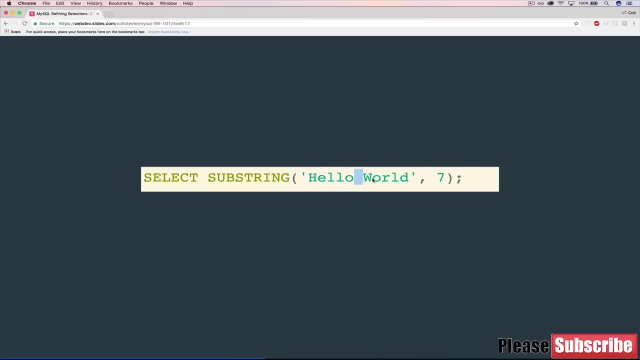 So if we count One, Two, Three, Four, Five, Space Is six, Seven. Is that W? You might think it's only going to give us that W, But it gives us From that W On to the end. 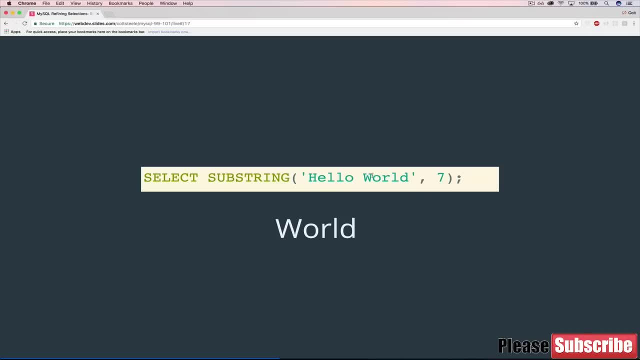 So if you only pass in One number Rather than two, It starts from Whatever that index is And just goes to the end. So let's try a couple out. We'll do a select Substring And we'll just do the hello world example that we just saw. 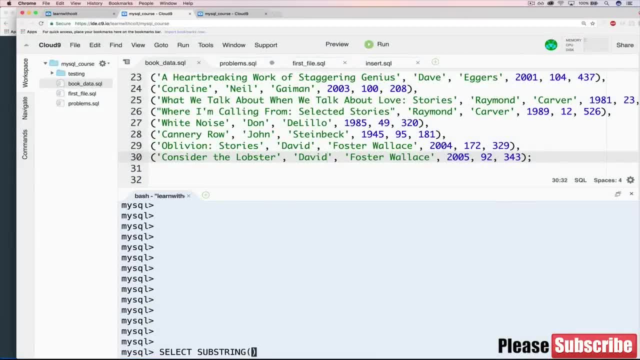 And we'll go from one to four. So we already know the answer here. Oh, There's hell, As you can see. One, Two, Three, Four, We get hell. So One, Two, Three, Four, We get hell. 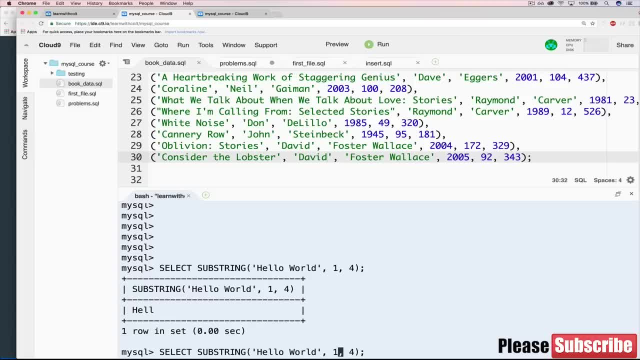 So if we change that From Let's do three To eight, We get Low World. So that's one way of using it. And then the next way, As we saw, Is if we just Leave that second. 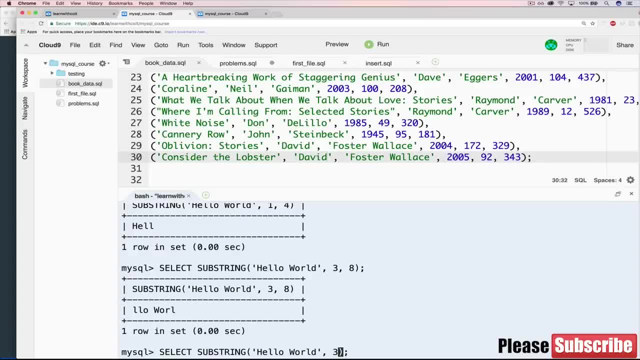 Or that third argument off And we just say Hello world, Comma Three. It will go from the third character, So one, Two, Three To the end. So we get Low world. Or in the case that I showed, 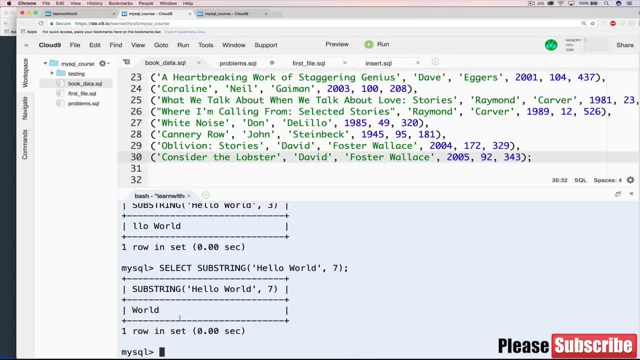 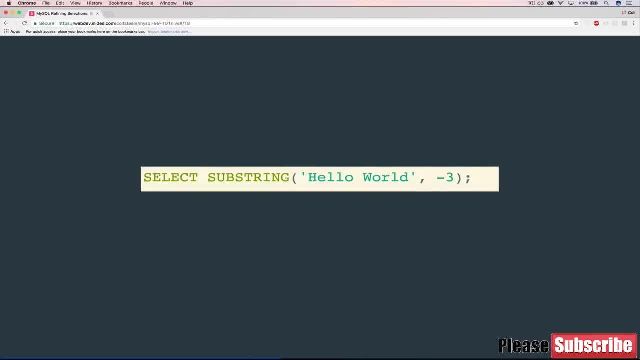 If we do seven, We get World, So Three. And there's one more way That we can use it, Which is to actually give it A negative number, A negative index. So what do you think will happen? I give it negative three. 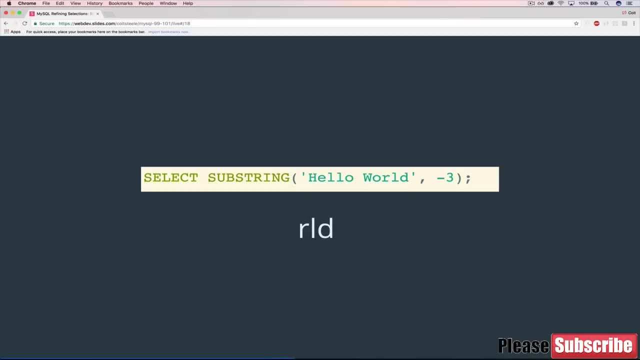 Hello world. Well, The answer Is that we get R L D, So it starts from the end of the string And it goes from One Or negative one, Excuse me- To negative two, To negative three. 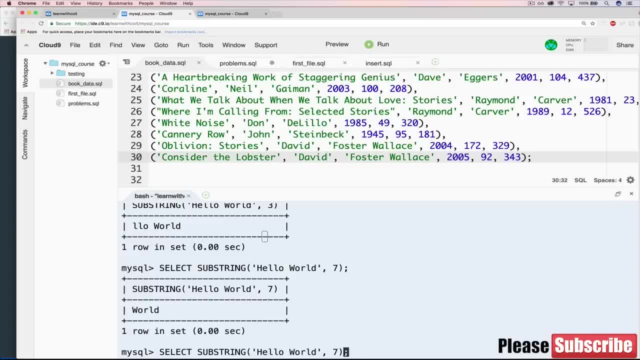 It includes all of them, So R L D. If we try that, Give negative three, You can see We get R L D, And if we did Negative Seven We'd go One, Two. 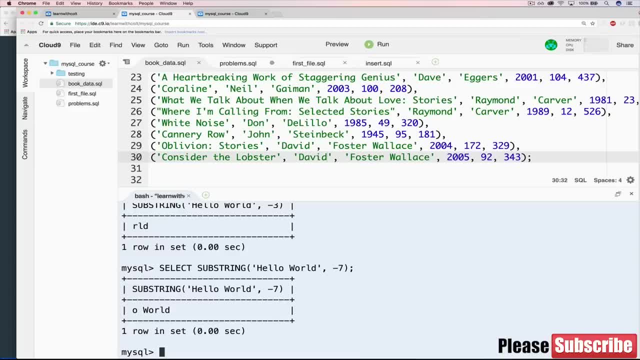 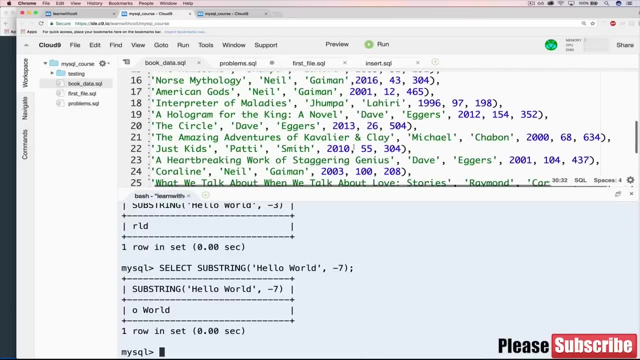 Three, Four, Five, Six, Seven To this O And we get O World. So that's how we do it With just Static datum. But now let's say We wanted to work with A column. 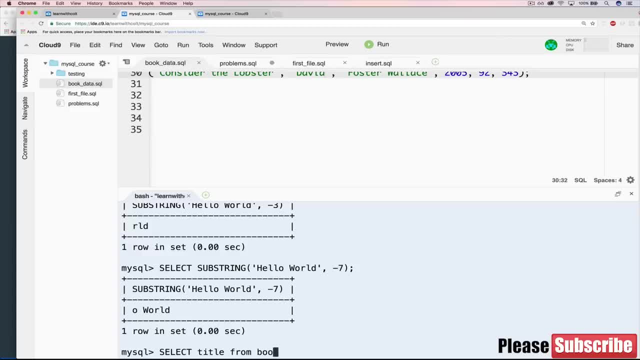 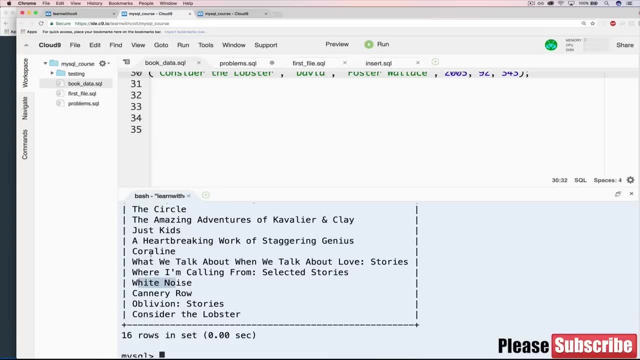 So in our case, Let's take the example- Select title From books. So we've got A variety of Lengths of titles: Right. Short ones Like white noise, Coraline. Long ones Like What we talk about. 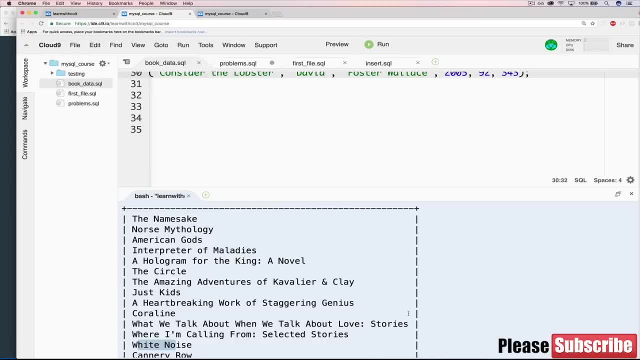 When we talk about love Stories, Let's say, I wanted to just print out- I don't know- The first Ten characters Of every title. Maybe You know, You've probably seen that before When you're on a shop. 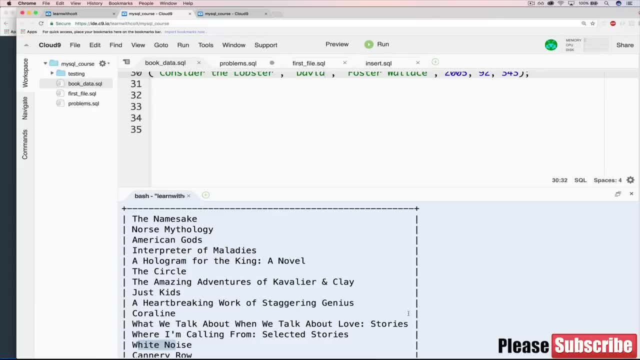 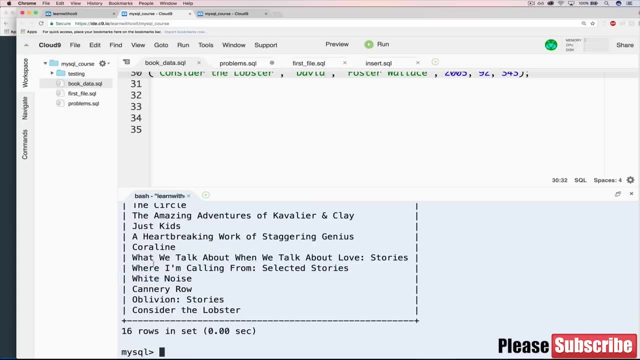 And if there's a long title, The whole thing Isn't printed out, There's just, You know, Something like that That you can click on. We'll do something similar. So To limit this, What we would do. 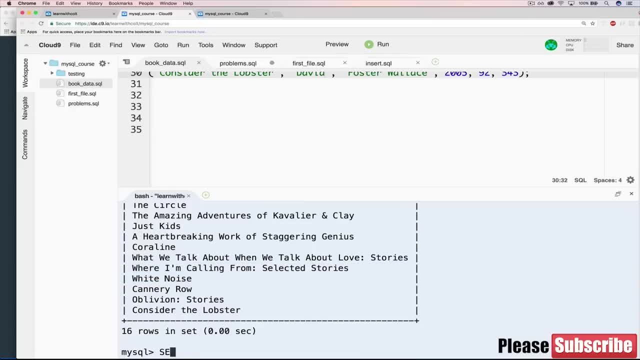 Let's just take this As an example. We can do A select Sub string, We'll give it The whole title, And then We only want From zero To ten, Or from one To ten. Excuse me, 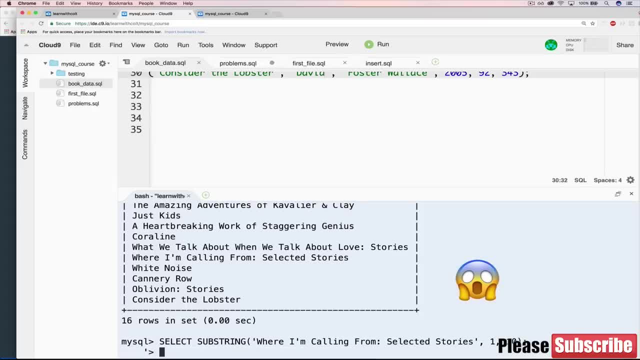 We could do that And this. Actually, Here's another error That I considered Editing out, But I've decided not to Because It is worth Taking a note of. The problem Is that It thinks That I'm still. 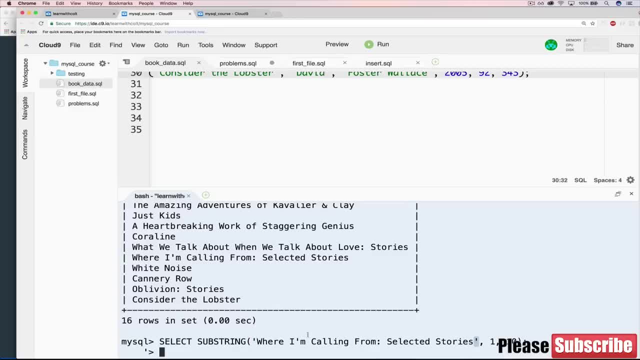 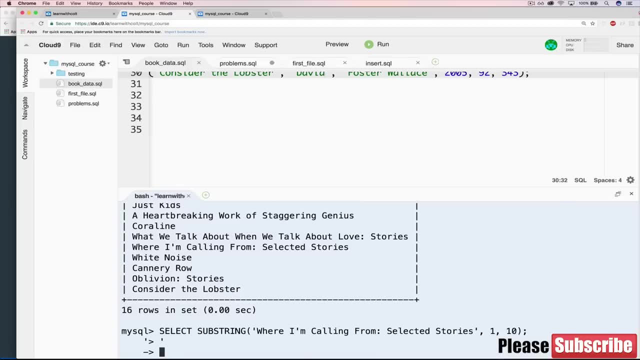 In a quote, Because I have this opening quote And this closing quote, But in between I have Another quote Which is actually an apostrophe In this case. So This is not Going to work If I do this. 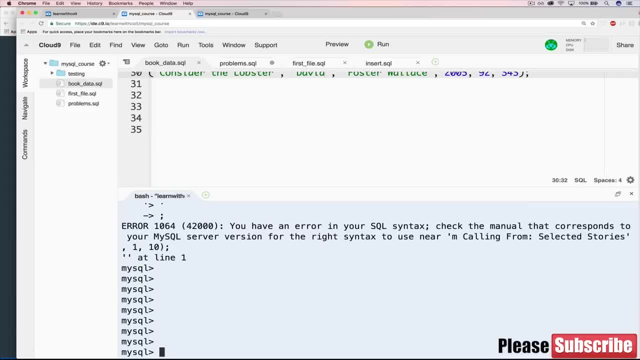 I'll just exit out, Just Ignore that, But I'll have to redo the whole line And rather than using single quotes, I'll use double quotes, Like this, Where I'm calling from Selected stories, Just like that. 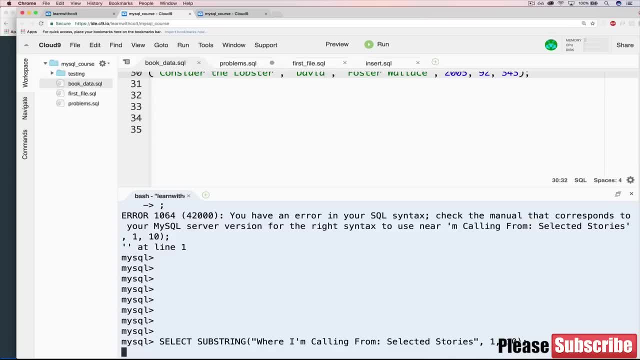 Alright, And then I'll get rid of this other quote I put at the end. So That is important. Just to take note of When we're working with strings. If you have A quotation mark in there, You've got to work around it. 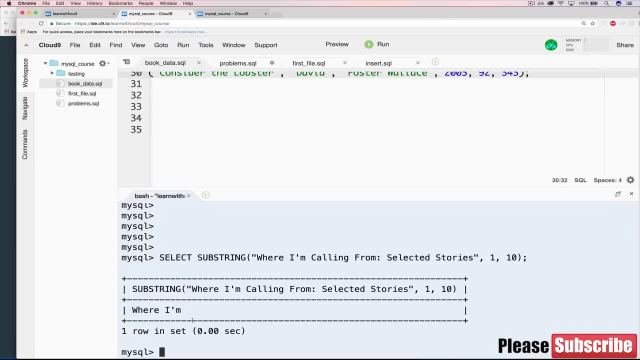 Alright, So I do this And you can see It gives me where I'm. Yes, This is 10 characters. Maybe isn't long enough, But we're just going to work with that, So We're going to do. 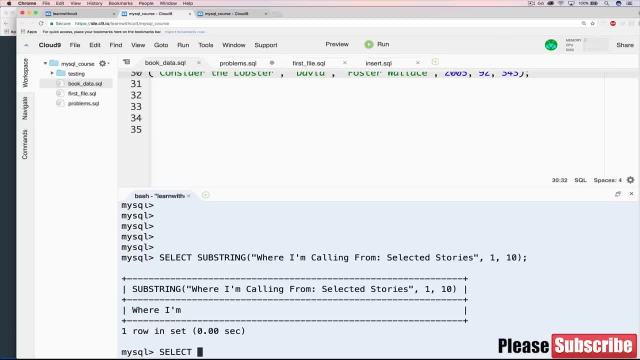 Every single Title. It works just like we did with concat. We're going to do a select Substring Title, Comma 1.. Comma 10. From Books, And that's it. And there we go. 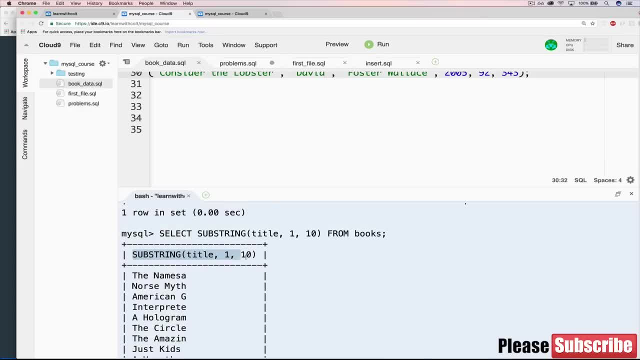 Now we have this ugly Heading up here, So we could do an As, Again, As, And, let's just say, Short title Like that. Okay, So That's it. So Now We get this Short title. 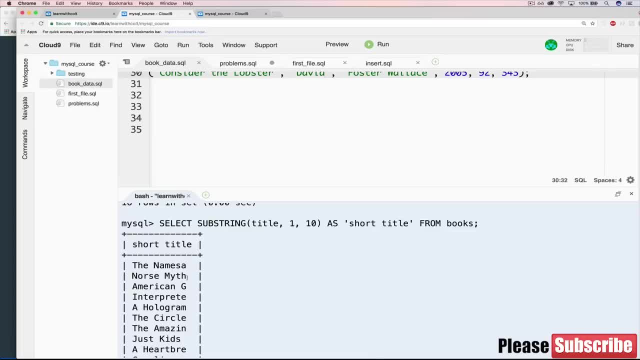 Blah, Blah, Blah. The name Say Norse myth, American G A hologram. Some of these actually work The circle. There we go, Just kid, All right. So One other thing I'll show you. 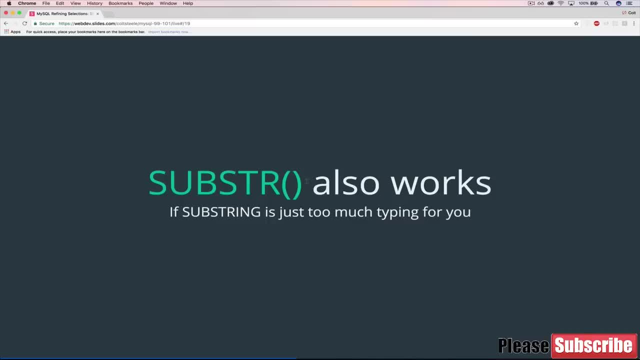 There is a shortcut. It's a very Small Shortcut, But you can type Substr, Substr. I don't use this All that often Because In some languages There'll be Substring Where it's. 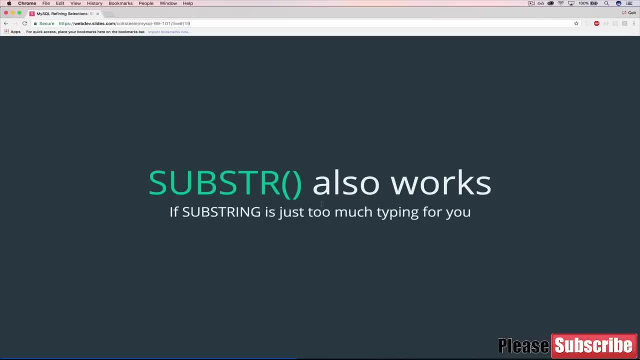 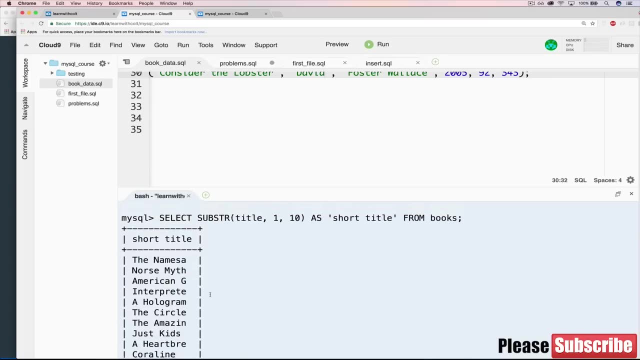 S U B S T. There's some. I've seen Where it's S B S T. It's just not clear Which characters Get cut out, Because it's not just All vowels, Because we have a U. 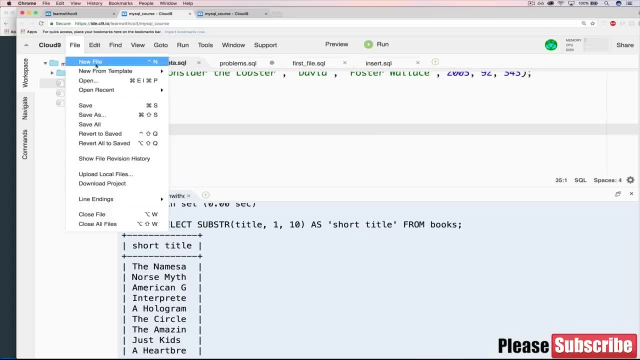 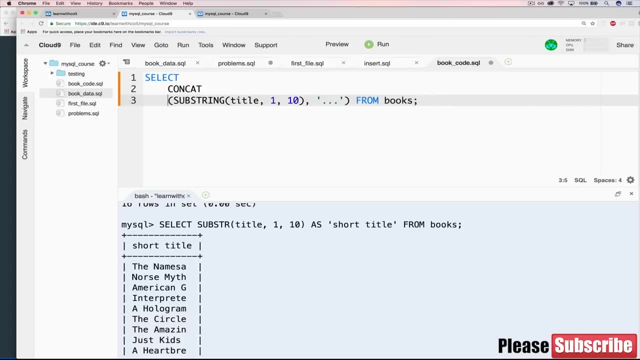 Still Anyway. So If you would like, You can use this. I can just show you If you replace that We do select Substring And just change Substring To be Substr. But what I also want, 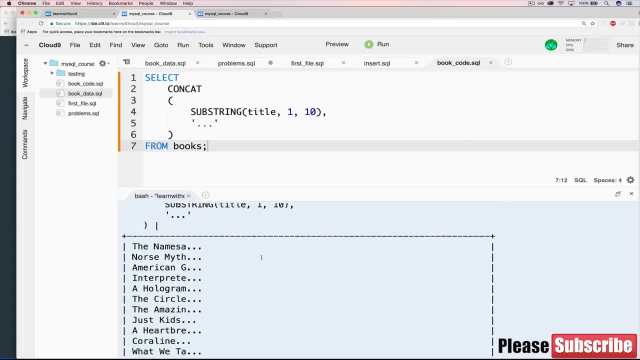 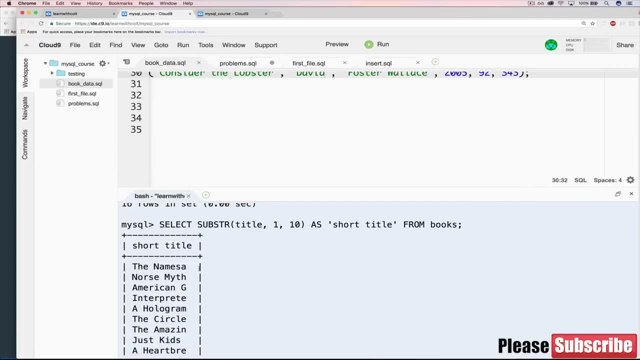 To show you Is that we can combine Concat And substring Or any of The string operators Or the string functions. You'll see. So let's say I wanted to add A dot Dot Dot After this. 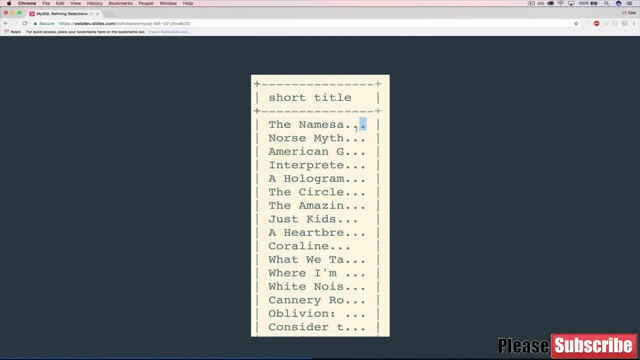 So that it looks like this Short title, The name say Dot Dot Dot. Rather than just An abrupt cutoff, Let's add a Dot Dot. So hopefully You can identify. What we need to do Is first: 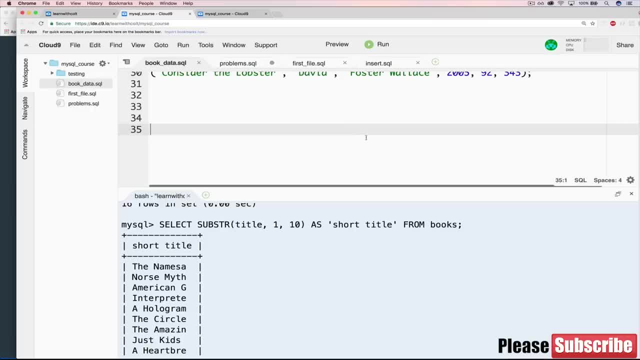 With Dot Dot. So I'll do this In a separate file. I'll go ahead And make a new file And I'll just call it Something silly Like Book code: Dot Sql. So we know. 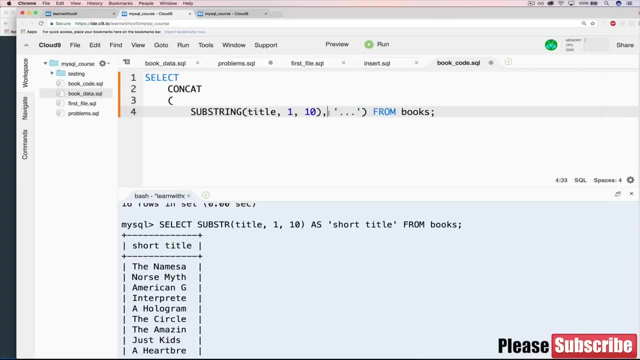 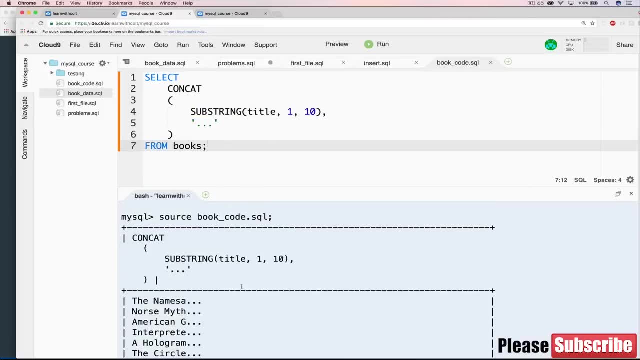 We're going to do A select And there's going to be A concat In there, And what we're going to concat Is the Short title. So again, This is wrong What I'm typing, But I just want to put. 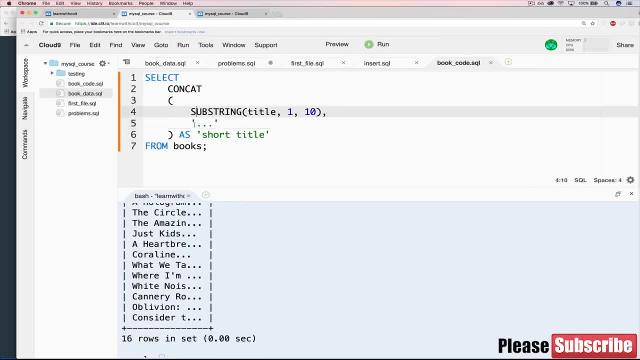 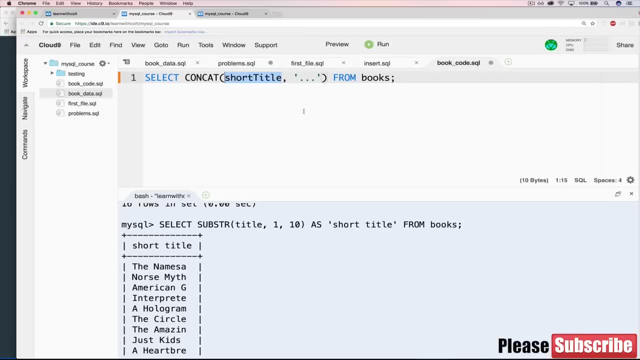 A placeholder The short title With Substring. We need to replace this With How we actually achieve That short title And that's going to be With a substring. So in here We type Substring And we want to put. 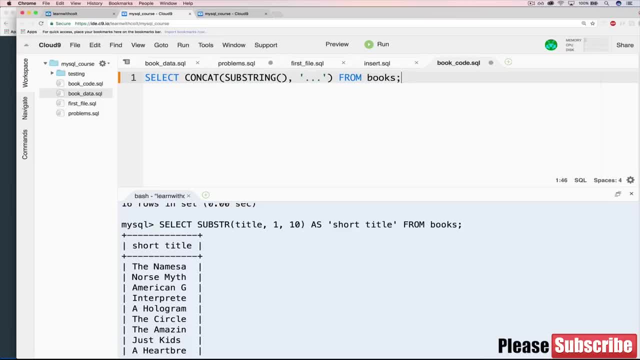 Title In there Oops Comma And we want it to go from One To ten, So this looks like a lot. It's pretty ugly. To format it A little nicer, We can do this. Depends on how. 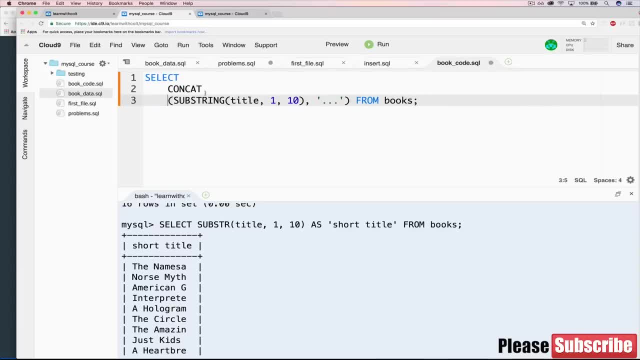 Intense You want to be About it. So this Looks like a lot To be about it. I like to just do it Like this Here. So substring Is our first argument. Comma Dot Dot. 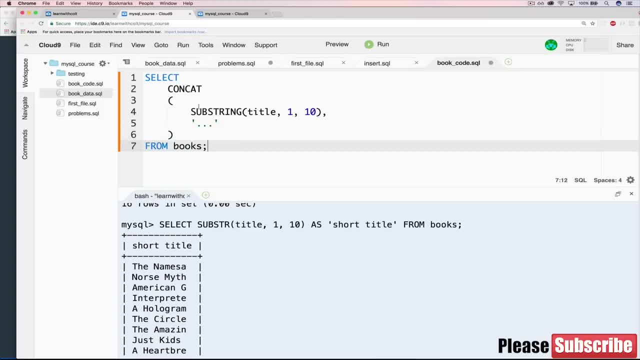 Dot Is our second one From Books, So if you look at it You can see The order Things are going to happen. So Substring Is going to happen first For every title. So that will be. 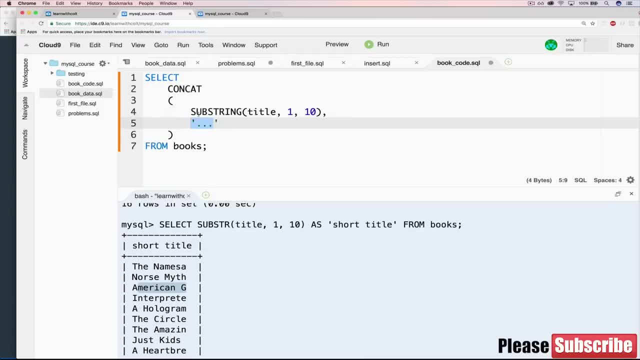 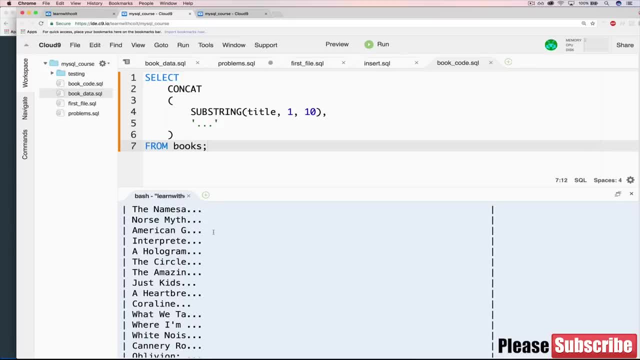 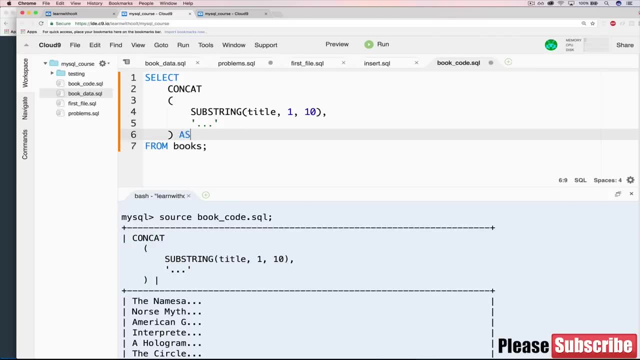 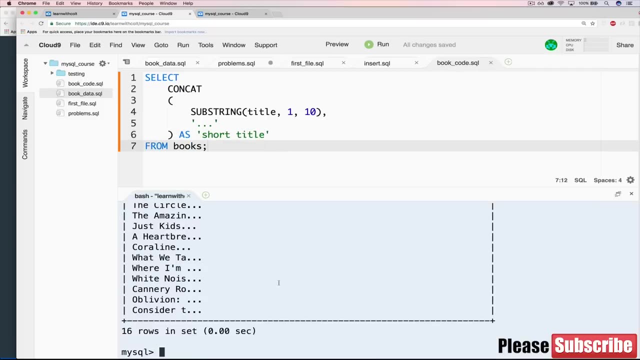 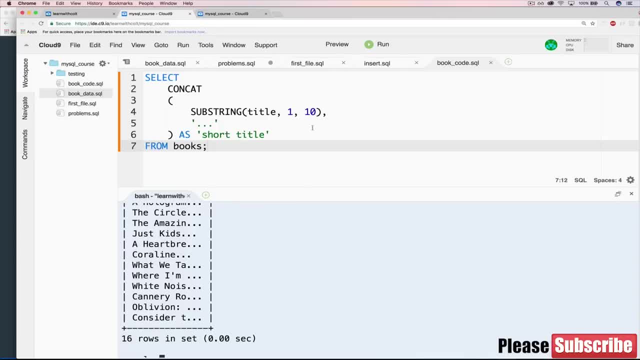 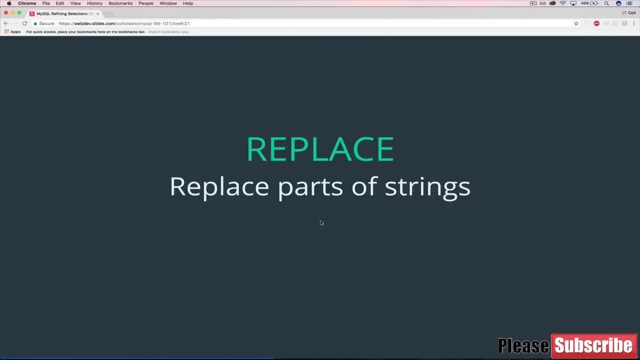 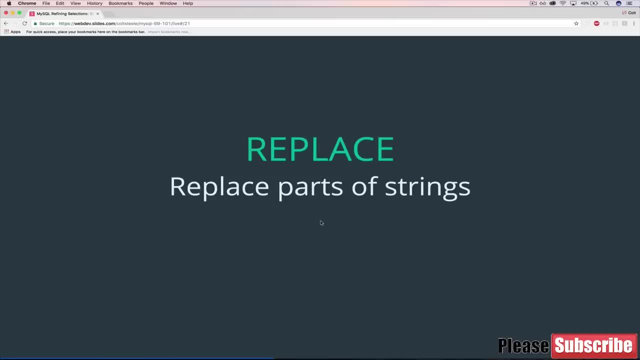 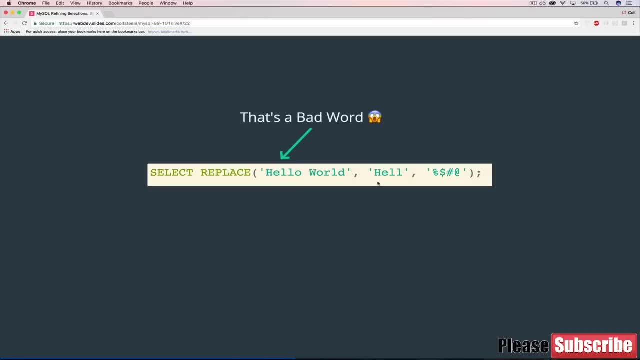 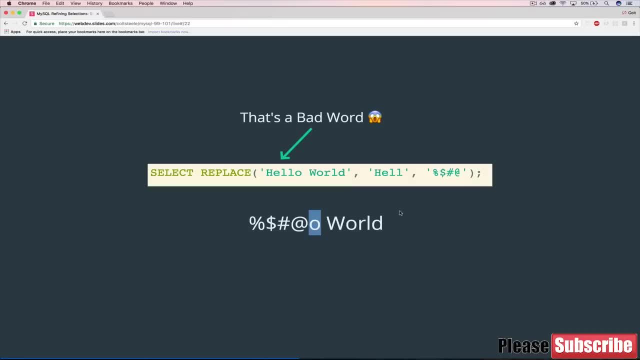 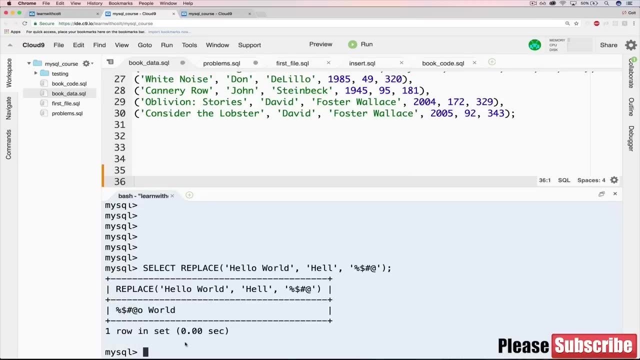 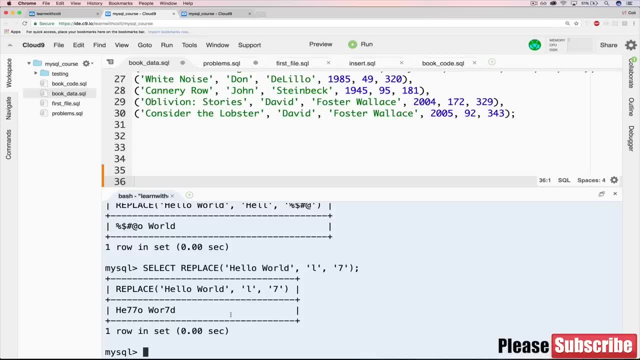 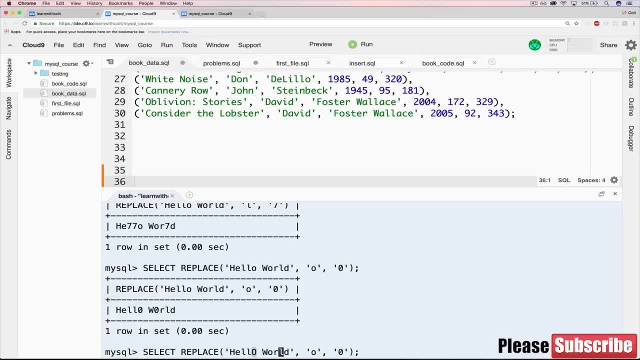 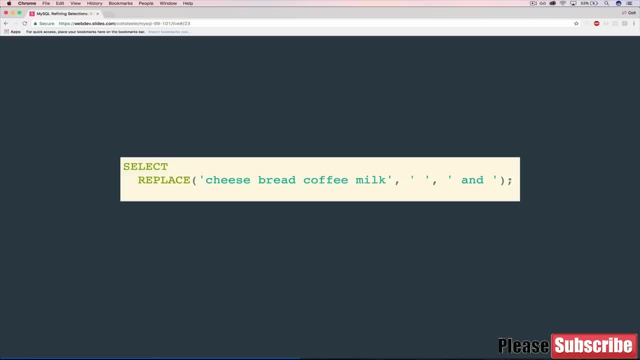 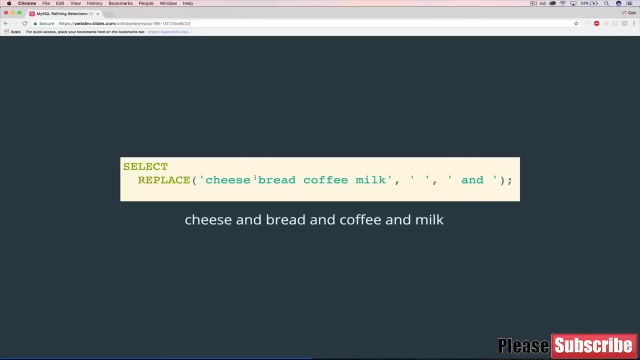 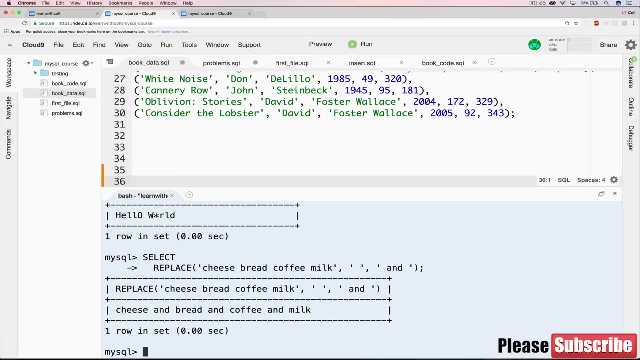 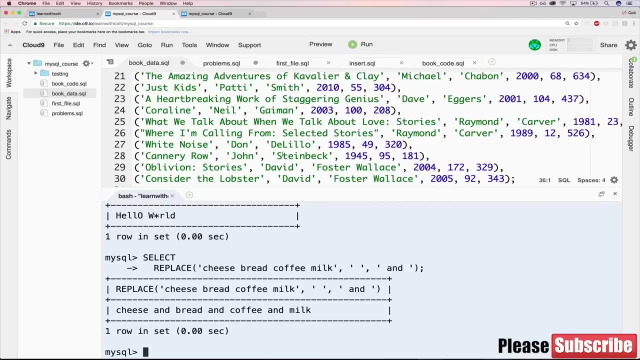 milk. it inserted that right there, here, here and here every time there's a space. so if i try running that, you can see it works: cheese and bread and coffee and milk. so now let's do something with the book data we have. we'll do something really simple and similar to what we just did. let's 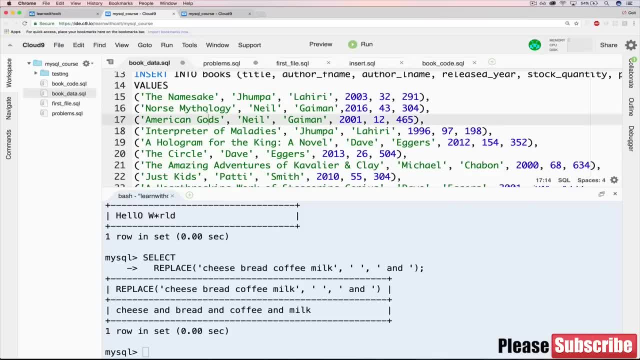 replace all e's with threes and we'll just do lowercase e. so anytime there's a lowercase e, like namesake norse, american, we'll replace it with a three. so to do that is a select replace and don't ask why it's not really. 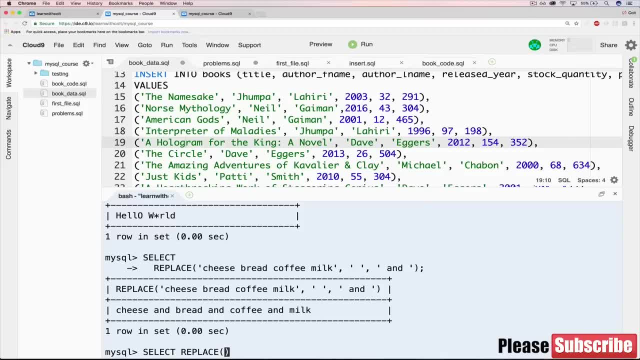 you, uh, a real world example. but select, replace you want to do title. and then what are we trying to replace? lowercase e's, what do we want to replace them with? three? and then what table? from books, and we could get more specific, but let's just do from books. 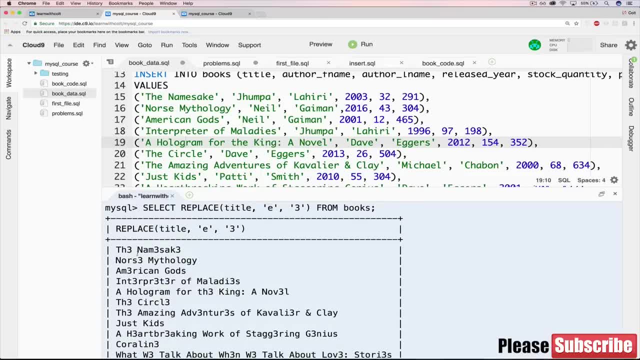 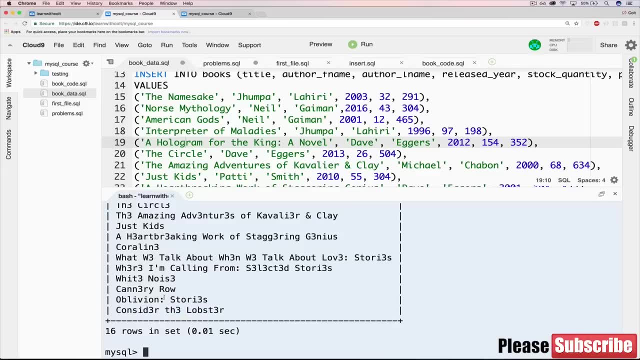 and you can see we get the namesake with three, threes and all the way down. consider the lobster, canary row. and so, and that's pretty much it to using replace. a bit of a bonus at the end here is that i'll show you we can combine replace with other functions. like we've already seen, we use concat and substring. 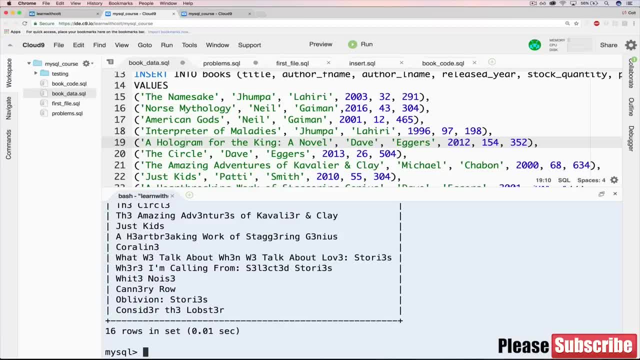 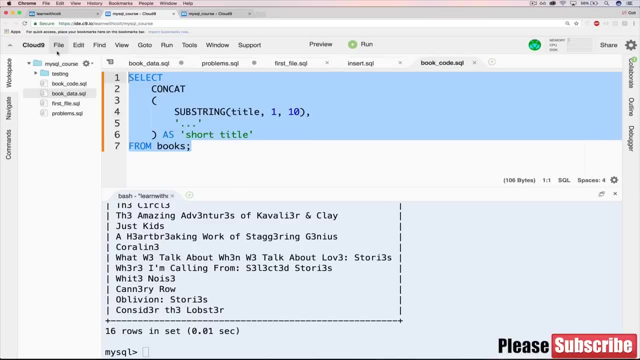 together so we could try the same thing by using replace and concat, for instance. so i could do something like: if i work in this book code, i will comment this out, which i haven't shown how to do yet: highlight it and on a mac it's command slash, on a pca, believe it is control slash, and then i'll. 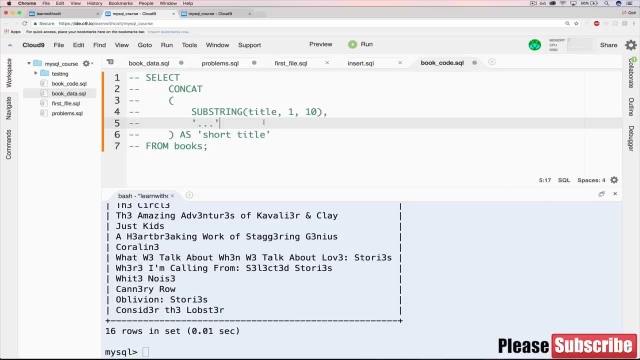 comment it out, which means it just won't run. it's here, so i can see it, but sql treats it, or mysql treats it as if there's nothing there when it runs it. so what i want to do now i want to combine, replace, so what i'm going to do is select and i'm just going to fill in the some rough blanks here. 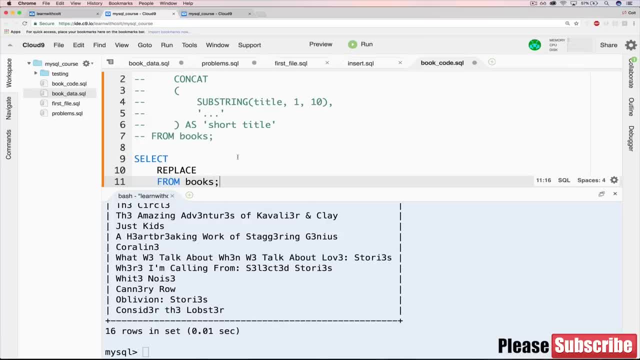 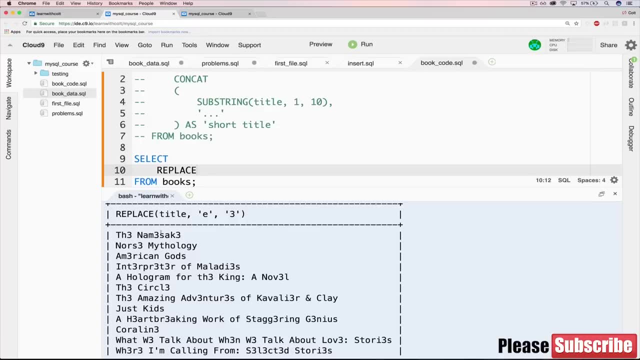 so we have replace and then we're going to have from books. but what we want to do is not just replace things. i'll do the same thing where we replace the books and then we're going to have replace all e's with threes, so that's replace title. 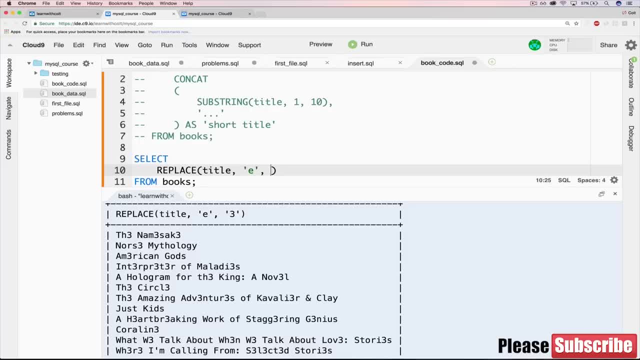 the lowercase e with three like that. but i'm only going to take the first 10 characters, like we did with substring. so i need to do substring and i want to do substring of this whole thing and you know, i'm realizing that i'm not going to be able to do that. 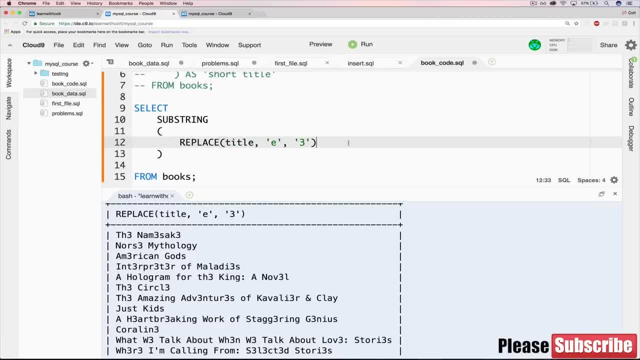 but i'm realizing, as this goes on, this is a little convoluted, so i'll throw up another. don't panic here. this is more just me showing you that it's something you can do, but it's not essential that you wrap your head around this entirely, but just to show you. so. substring and the first argument. 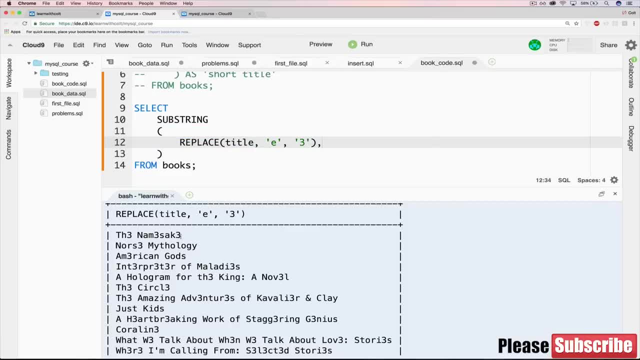 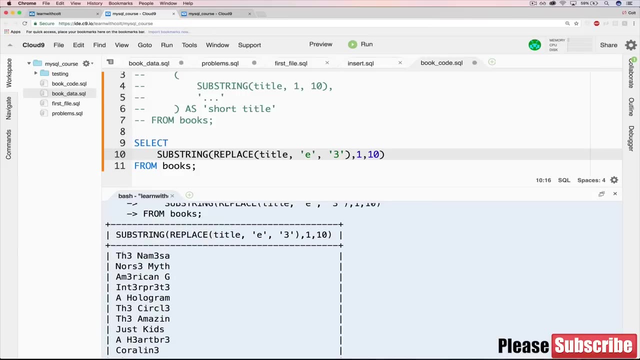 is replace this whole thing. so basically we're taking a substring of this and then of this and we want to go from one to ten. so that's a lot there. and now, if i paste it in here you can see, what it did was first replace all e's with three and then take it the substring of that from one to ten. 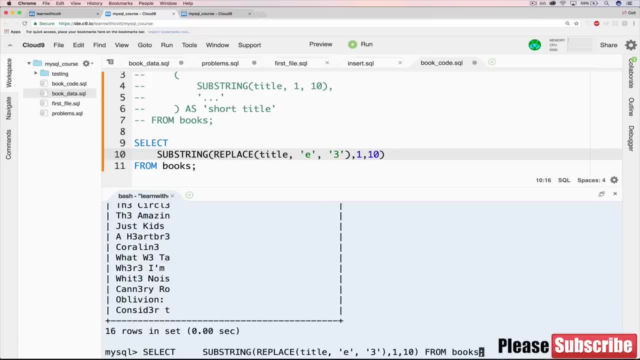 and of course we could give it a better name because it is pretty ugly. so we could do as weird string, let's say: and now we have weird string up here and yeah, that's pretty much it. i just wanted to show that we could combine them together. 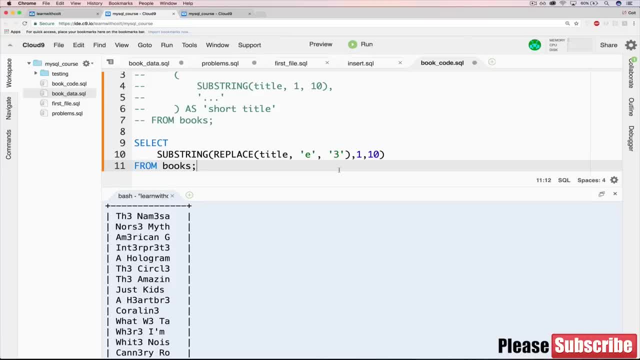 Why you would do this exactly again. You probably wouldn't. but the key here is that they're kind of like Lego pieces. you can Reorder them. you can Well, maybe more like nesting dolls actually, where you can nest them inside of one another. So like we did substring inside of a king cat, we can do a replace inside of substring. 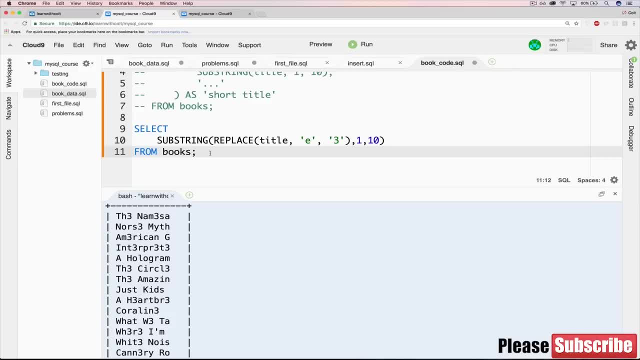 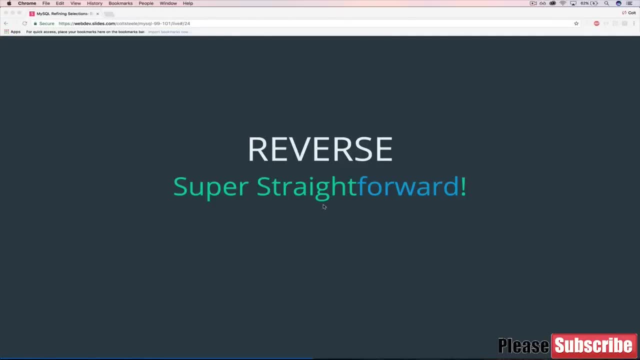 So that's enough of replace. We're gonna continue with a couple more and then we'll do some challenges. All right, moving along to the next function, which is reverse. and Reverse does what it sounds like: it reverses strings. That's why I said it's super straight forward, you know: forward, reverse, It's a joke. 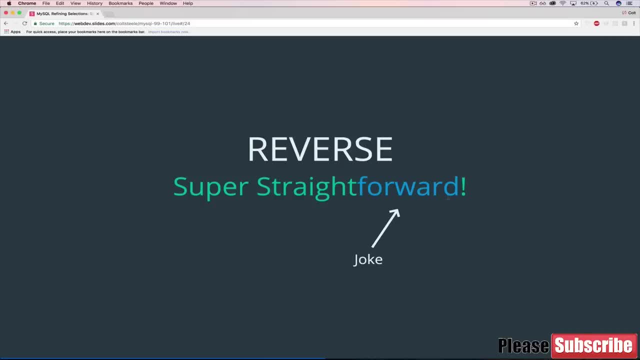 Yep, So that's what it does: It will reverse a string. so here's an example: select reverse of hello world and We get this: draw, Ola, ole. I think it's probably best if I just stop pronouncing them from here on out. but You get the reversed version of the string. same casing and everything, same space is just reversed. 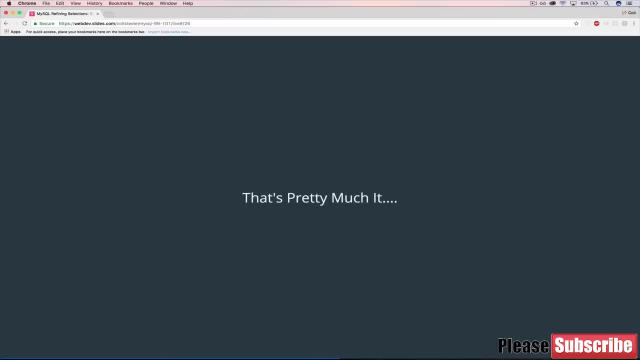 And that's kind of all there is to it, to be honest. I'll show you a couple examples, But if you feel like you already have it, you know That was enough for you and you understand how it works and feel free to just move on. But I'll go over to cloud nine and show a couple of examples, So let's do a select. 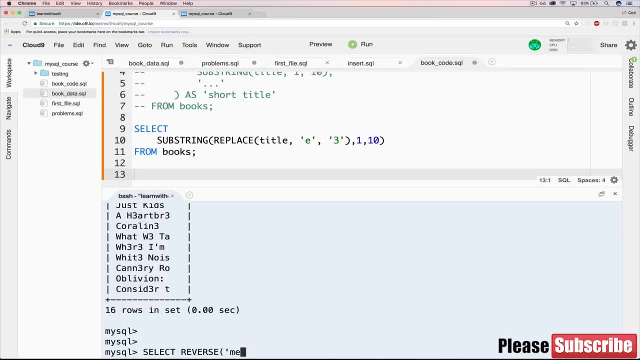 Reverse and instead of hello world, Let's just do meow Meow Meow. why not just like that? and We get what? oh, I said I wouldn't pronounce them. Well, we get this right here: Reversed of meow meow. so we could do the same thing to find the reverse of. 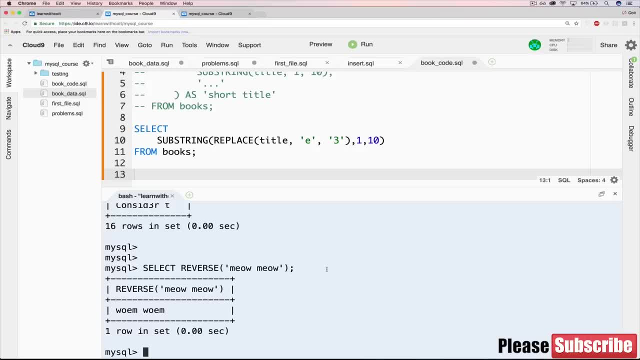 Every author's first name in our table, for instance. so that would be a select reverse Author F name and then from books, And there we go. We get the reverse of jumpa, the reverse of Neal, and so on, and that's kind of it. and 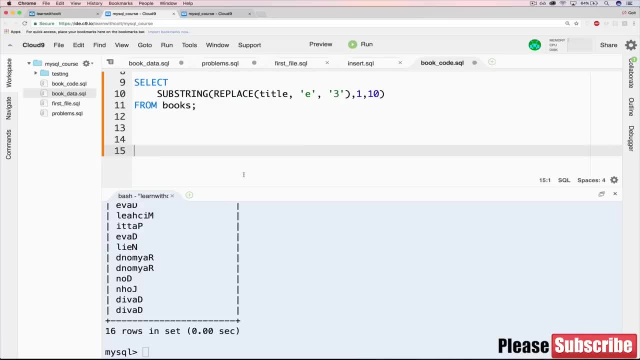 Just like some of these other ones, we can combine them. so if I wanted to turn something into a palindrome, for instance, let's say I started with the string wolf and, If you're not familiar, a palindrome, something that reads the same forwards and backwards. So the way I would do that is by adding F O O W to that. 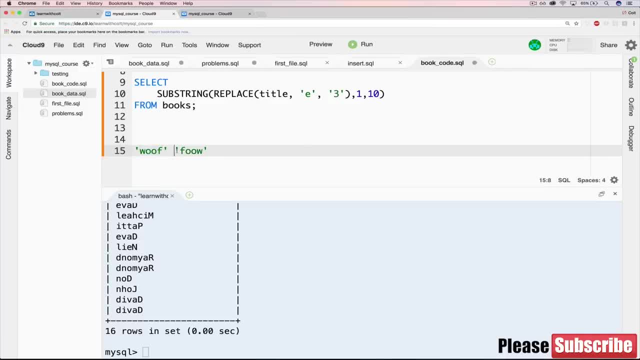 And concatenating them. so taking the original string plus the reversed string and Concatenating them. so we have two functions. We've seen how to do that and it's just a matter of can cat. so a select Can cat and we'll just start with woof and 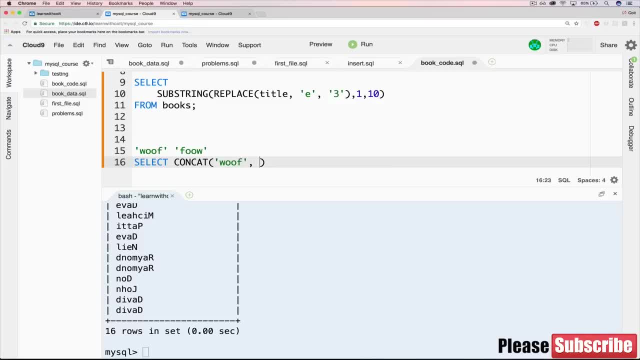 Then, what do we want to concatenate it with? Well, we want to concatenate it with the reverse of Woof, just like that, and That should do it. Let's try it out, and We get this, the palindrome version. I guess that we just made this sandwich. now Let's just try it with author's first names again. 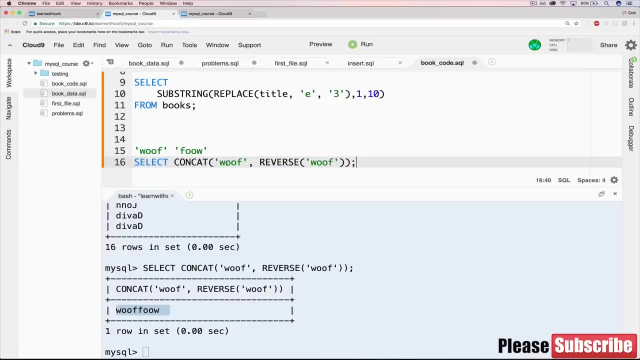 So let's do that now. All we need to do is replace a couple things in here. So, rather than Concatenating woof, we're gonna do author F name and Then we're gonna use the reverse of author F name as well, Just like that. and 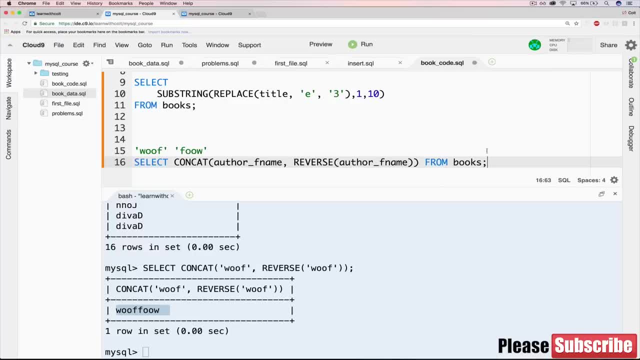 Then of course we need to say from where? from books. Let's copy that. so just again taking the author's first name, the reverse of the author's first name, and we're smashing them together with concatenating, and There we go. we get this one's kind of funny, I guess. David diva D. 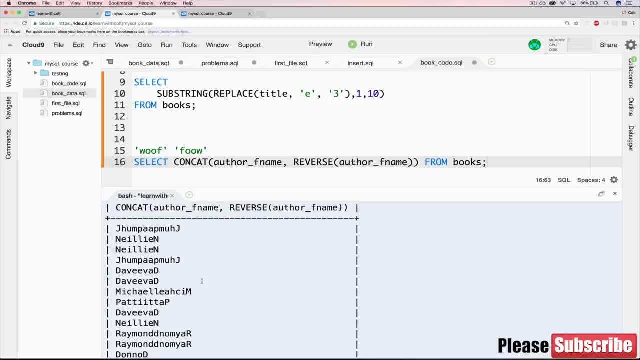 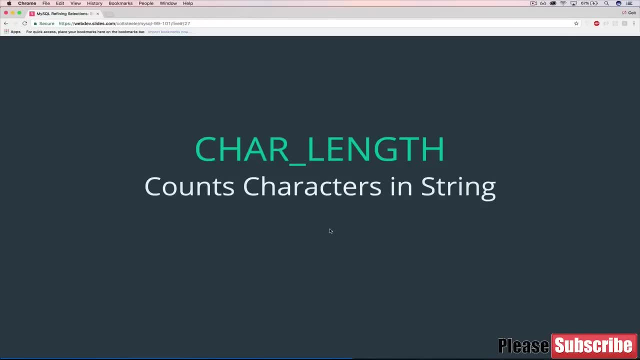 and I don't think any of them are really pronounceable otherwise, But they are valid palindromes, So I guess we succeeded at something. the next function We'll take a look at is pretty quick as well. It's called char length and what it does is it just tells you how many characters are in a given string. 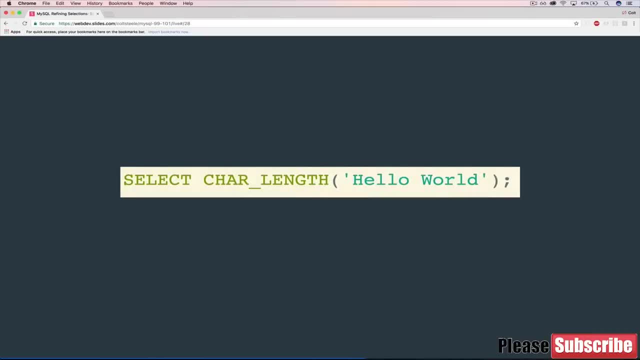 And that's pretty much all there is to it. So it looks like this Char underscore length and when we do it on hello world We could count the characters. so one, two, three, four, five, six for the space seven, eight, nine, ten, eleven, and We get eleven. at least my slide says we get eleven. Let's verify that. can't trust those slides. 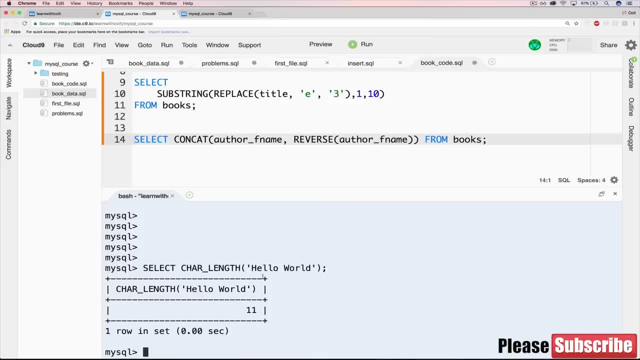 Whoever made them, Me. so you can see we get eleven. So if we changed it and just added a bunch of stuff, we won't count it, but it says that's 31 characters long. Okay, so we could do something like select and Let's just print out the author. 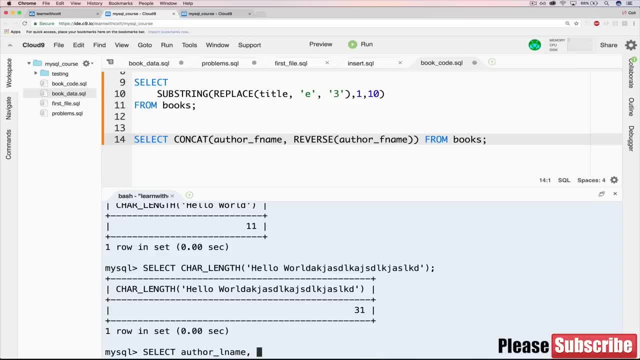 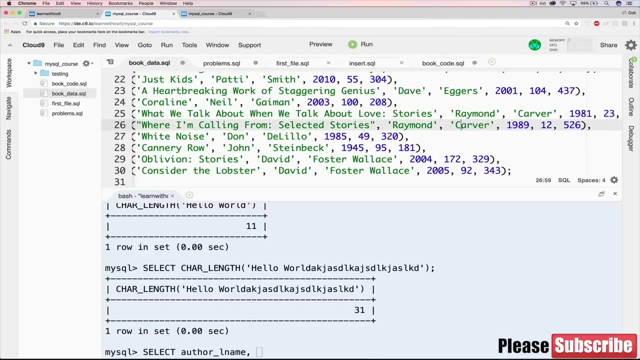 Last name this time, so author, I'll name comma. then we'll also side-by-side print the Chair at the character, the character length of the author's last name. So it might say something like Carver, and then next to that, one, two, three, four, five, six characters and Eggers, also six characters, and so on. 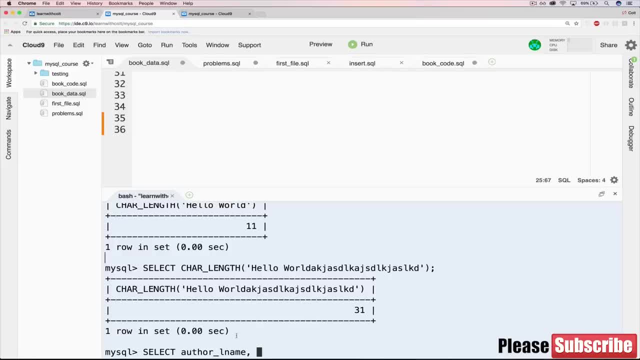 So it's just gonna be our author's last name, followed by the number of characters in their name. So character, char, length, author, l name, Just like that, and let's put an as here and we'll just call it. We'll just call it length, just like that, from books. We'll hit enter. 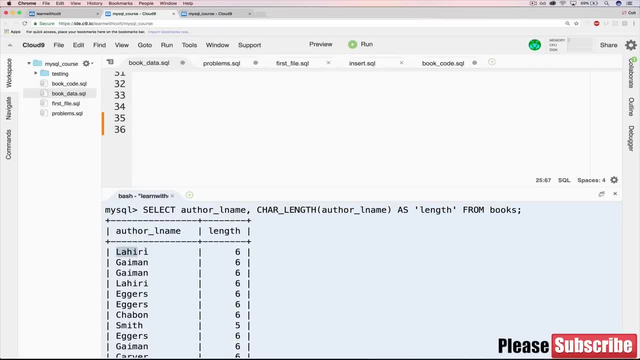 And you can see we get this nice little table with our author's last name and the corresponding length. so we've got a lot of authors who are six characters long, or their last name six characters long, and then You know we get Smith, who's the shortest, and so on. 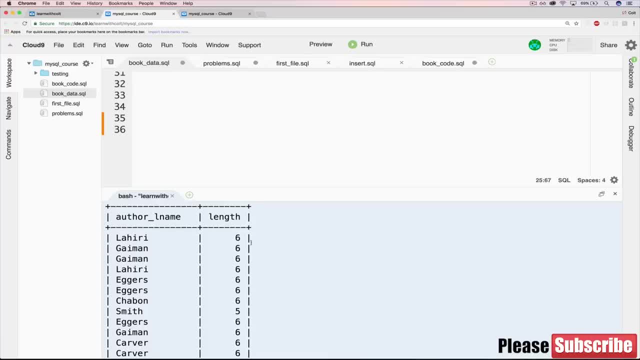 We'll see later on how we could sort things and order them differently, But for now we've got them all here, All right. So, just like before, if you feel like you have a grasp of this, feel free to move on. I'm just gonna show that we can also combine. 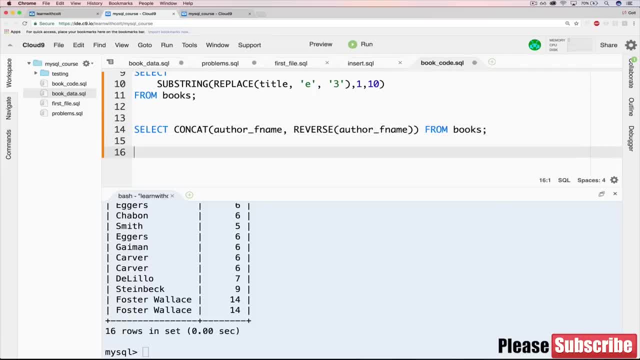 Character length. So what I would like to do is end up with a result that looks something like this: Eggers is, and then six characters long. So I'd like that for every author that we have. So if we break it down, this is going to be author's last name. 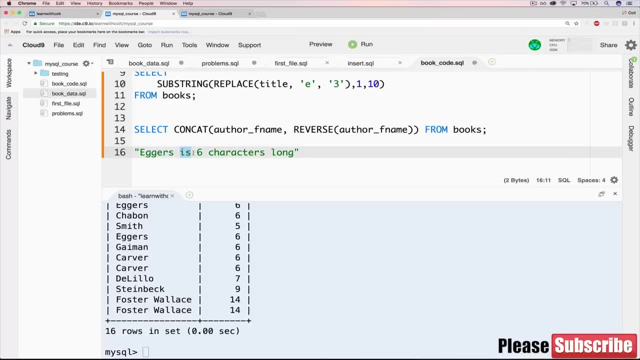 concatenated with is Concatenated with the character length, concatenated with characters long. So it's gonna be kind of a big one. So let's, let's try it out. We're gonna do a select can cat and, and The first thing we'll concatenate is the author's last name. 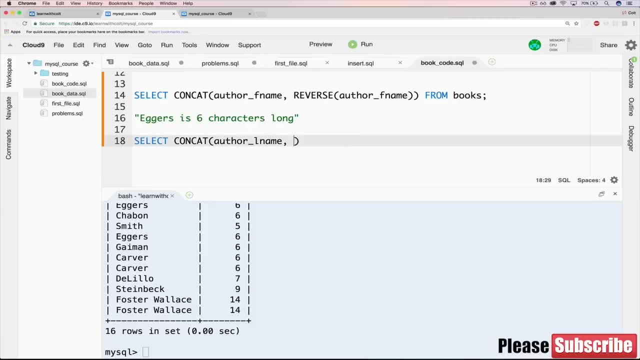 So author L name, and then we're going to concatenate that with space is Space, so that gives us this right here. then inside of that we're going to add char length of Author L name. you can see this is getting kind of long. comma is a comma is. 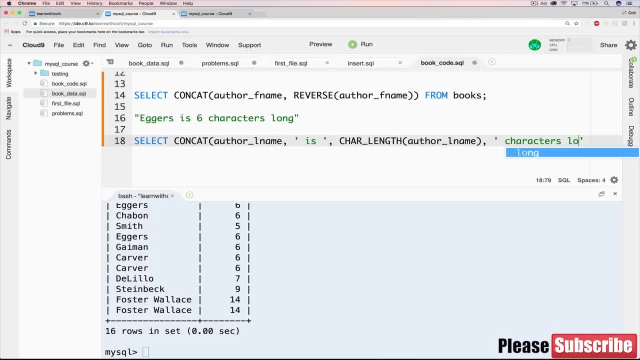 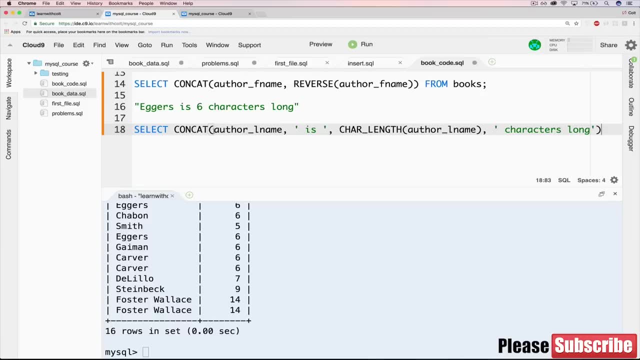 not is space, characters long and our parentheses. So that's kind of a lot. here We're concatenating the first thing- the author's name- and then adding is, and then adding the character length and then adding characters long. So we're building this sentence one piece at a time and then we also need to specify from: 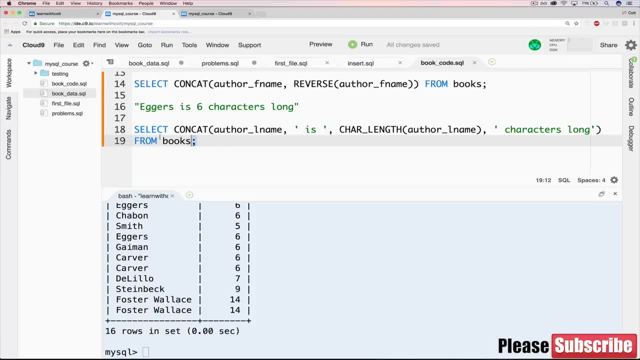 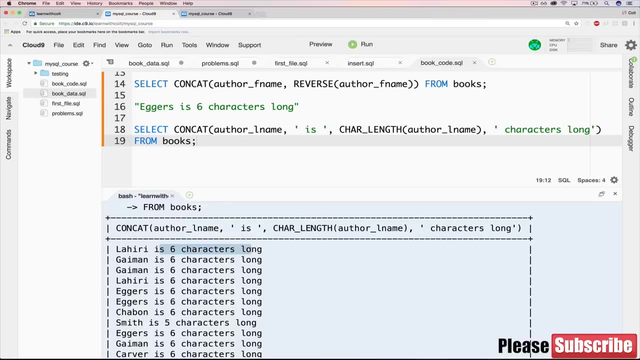 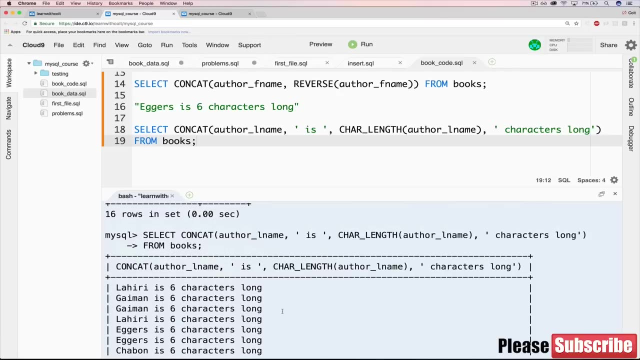 books. Okay. so let's take a look, let's copy this, paste and paste this in, And there we go. lehiri is six characters long, carver is six characters, steinberg is nine characters. foster Wallace is fourteen characters. So that's working. by now. 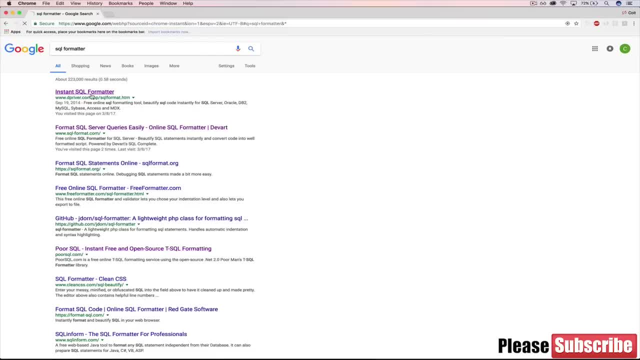 You should know we can use ads to make this a little prettier. The only other thing that I'll take a moment to address is that this is kind of ugly, Something that I do often- to format my sequel meaning is: use one of these formatters. 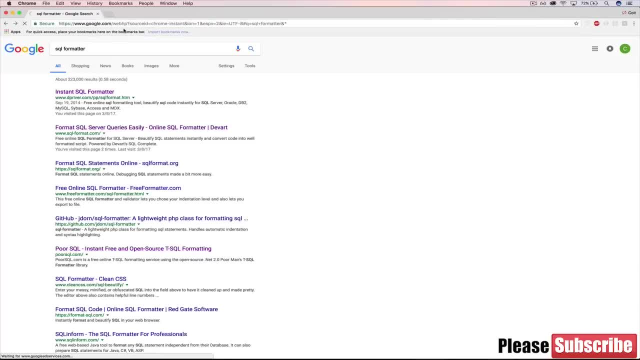 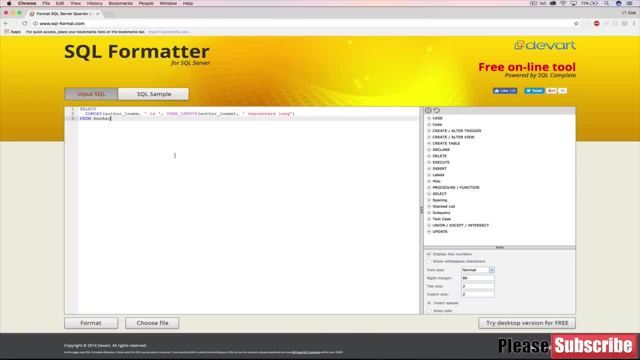 So there's a couple of them. I like this one, sql-formatcom, And I can paste in my query and just click Format And it will just format it a little nicer for me, And it depends on, you know, when things get really long. 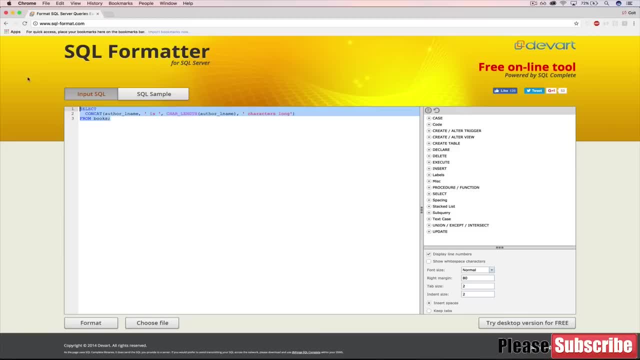 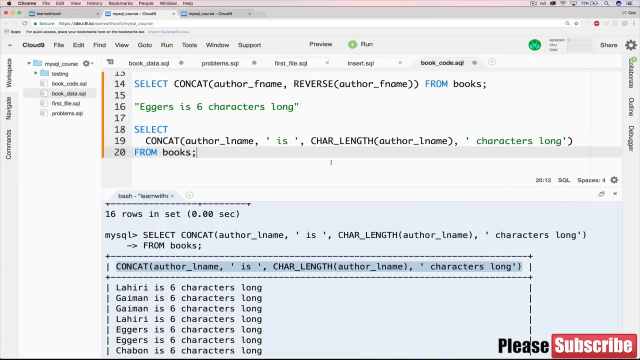 when you have long, create tables. it will clean things up nicely for you. So in this case, this is a cleaned up version. Not that much of a difference, to be honest, But we can replace it anyways. It's a little easier to read. 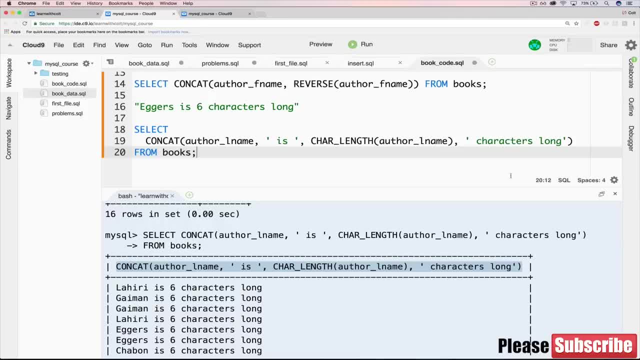 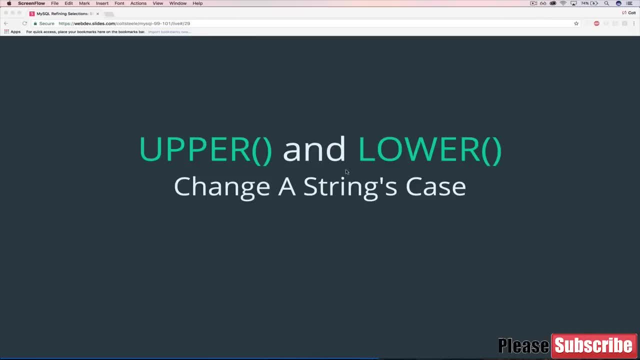 All right. So that's all there is to character length. That's all there is to char length. All right, Welcome back. So we've made it through a lot of string functions. We've seen concat and replace and substring and reverse and char at. 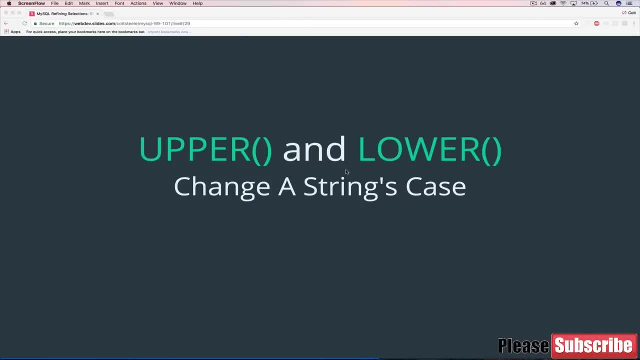 We have two more that I'm combining into one video because they're really simple and straightforward And they're a natural pair, And then, after we finish this, we have some fun exercises. So the two that we're looking at are upper and lower, and they do what they sound like. 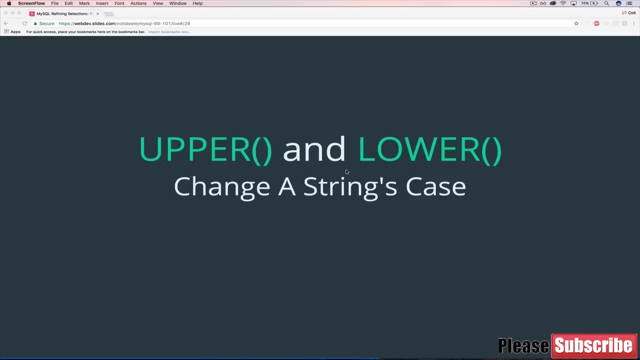 They change the case of a string so we can make something all caps or all lowercase letters. So let's take a look. What do you think this will do? By now you should be familiar with this select and then some string function. So select upper hello world is going to convert hello world to all caps. 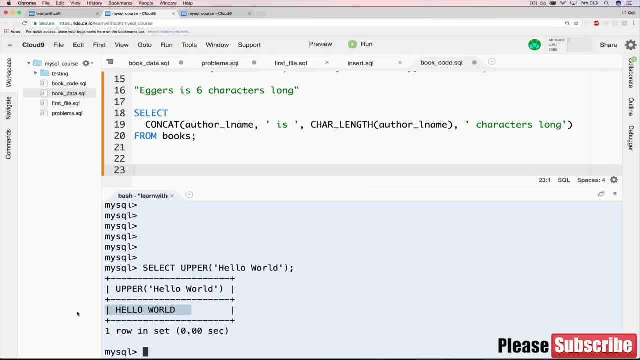 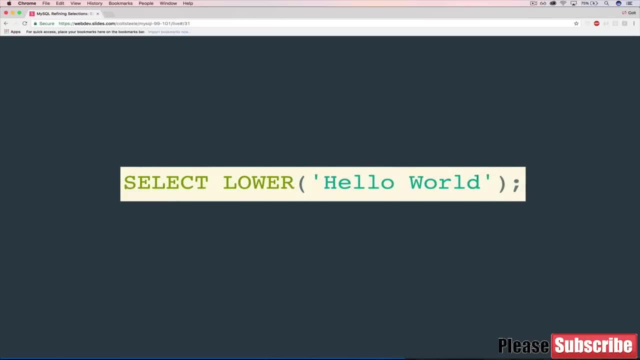 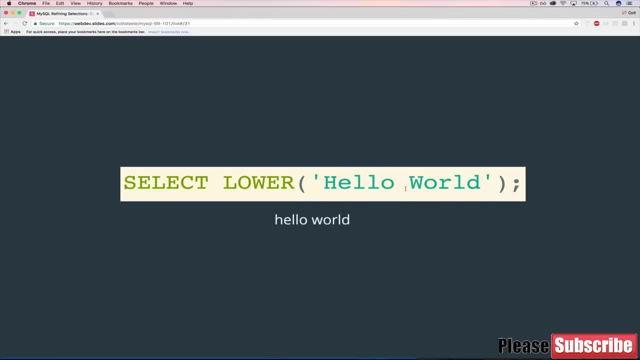 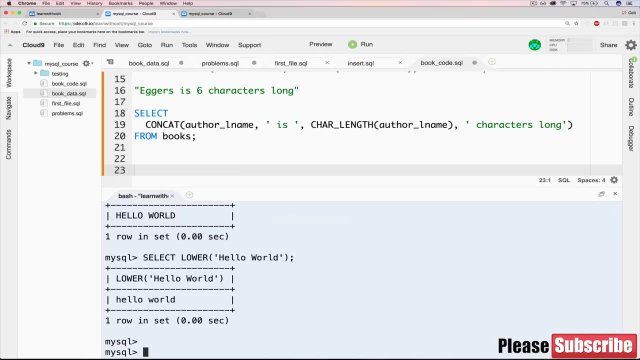 So it's really just the H and the W And we get hello world. Still don't believe me? Okay, There we go, Hello world. So, honestly, that's pretty much it, Just like the other couple videos before this, if you feel like that's good enough. 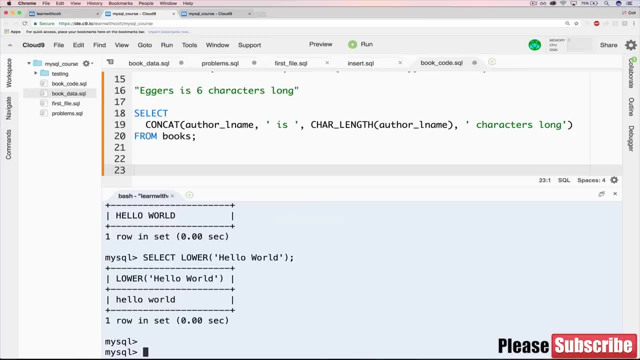 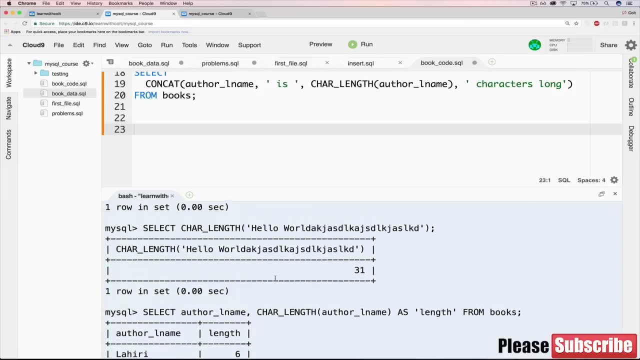 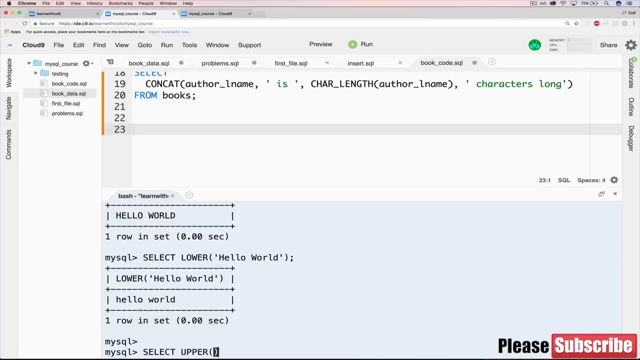 go ahead and move on to the exercise. But if you want to see me use it with some of our author data, stick around. So let's do something silly like print out, um, all book titles in all caps, So to do that it's just a select upper title from books and that's it. 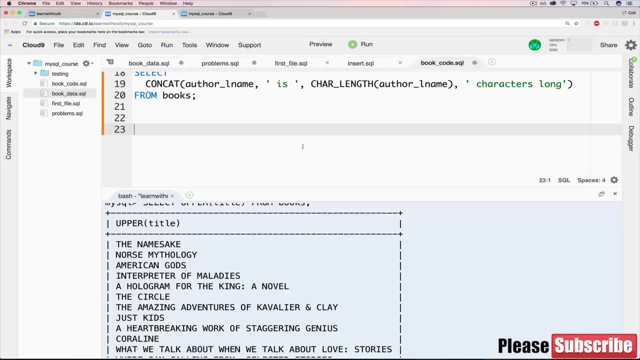 And of course we can combine it with other things, So we could do something like my favorite book is, as if someone was yelling my favorite book is, and then a book Name like the namesake, And to do that we need to combine the uppercase version. 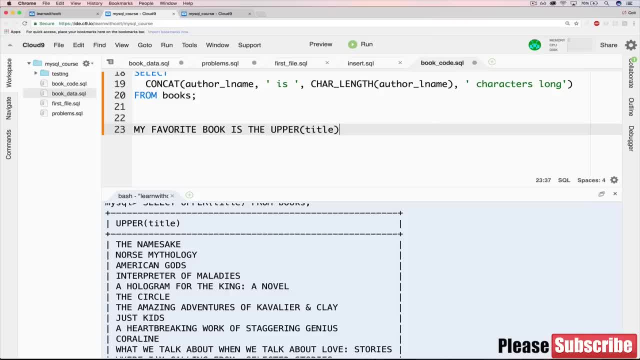 So I'll start writing it here: upper title, and we need to concatenate that with this string right here And to concatenate them kind of building backwards. here we need to use can cat just like that. So can cat my favorite book is, and we should add a space, the, and then the uppercase version of title. 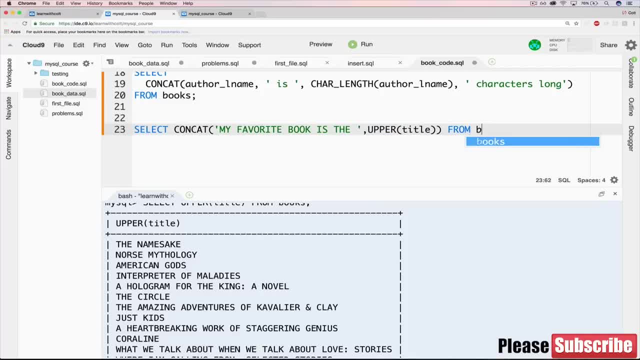 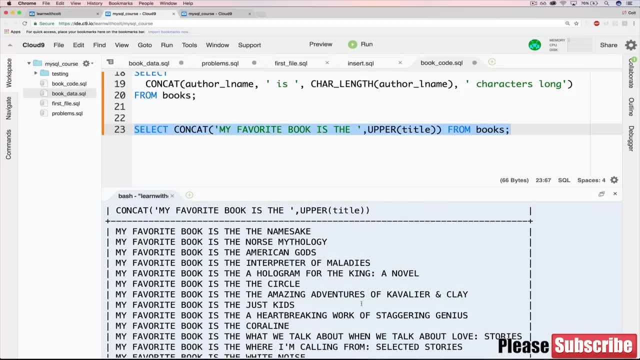 And then we'll just add a select can cat from books. So I kind of built that one in a different way, starting from the inside out, but you can see we get. my favorite book is a namesake, My favorite book is a circle. 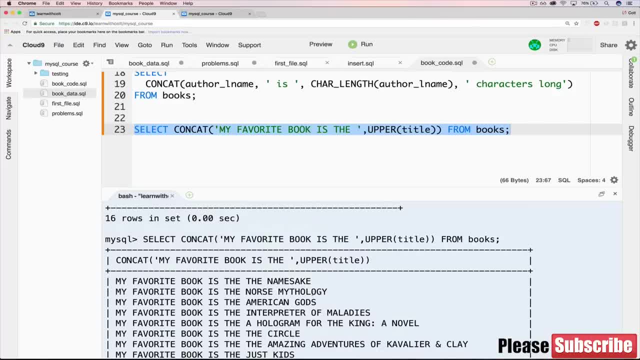 My favorite book is: oh, is the canary row? Yeah, I'm not sure why I put the the there. Whoops. Well, anyways, if we delete that extra the and rerun this Now, it's grammatically correct. 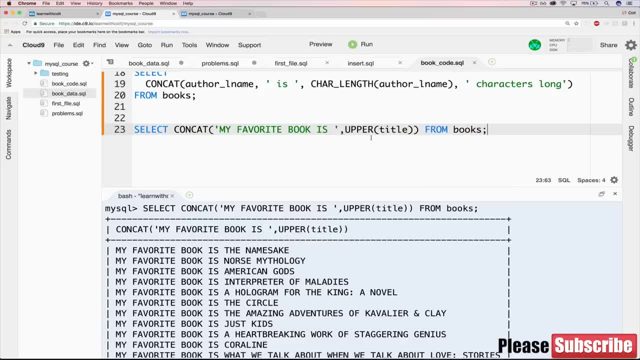 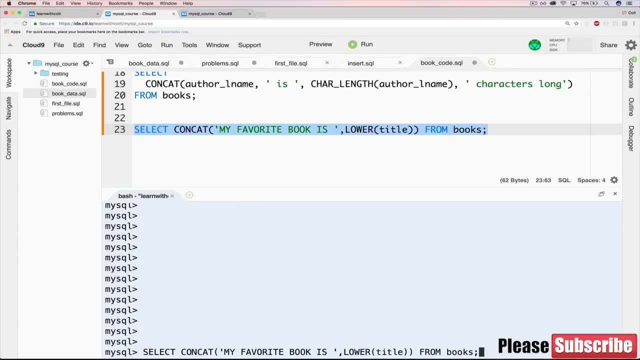 Um, so that's pretty much it to upper and lower. I mean we could change this to be lower, if I mean. fine, If you make me, I'll show it. I don't think there's any surprise about what will happen, but just in case, it just converts everything to lowercase. 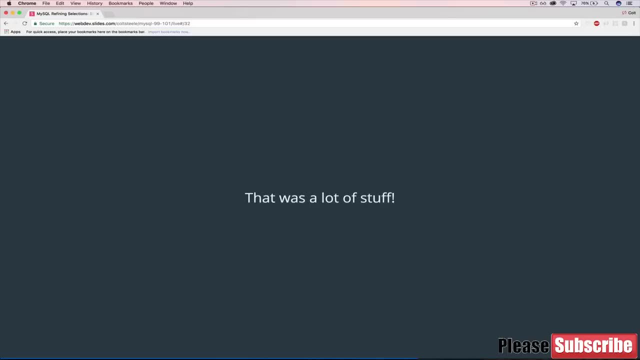 Okay, So that's upper and lower. That was a lot of stuff, all these different string functions we saw. Now it's time for you to get some practice doing it yourself. Okay, So you made it to the end, Hopefully. I mean, I guess you could have skipped forward, but you made it to this video. 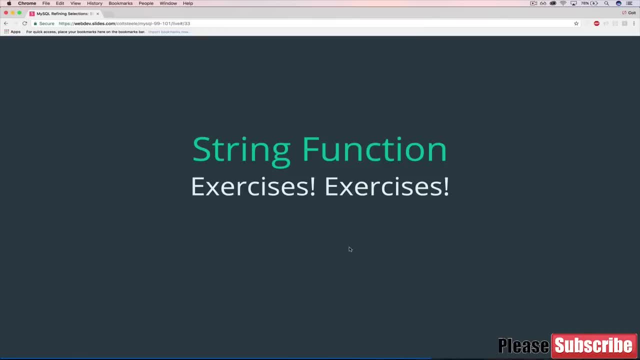 However, you got here, um, at the end of the string function section. So we have a couple of exercises- and they range from pretty straightforward to reasonably complex- where we combine multiple string functions together. So let's get started. The first one here is to reverse and uppercase the following sentence: Why does my cat look at me with such hatred? I would also appreciate an answer to that, If anyone can help me. uh, but anyways, what we need to do is just take this. You can copy it or type it out and just use my SQL. 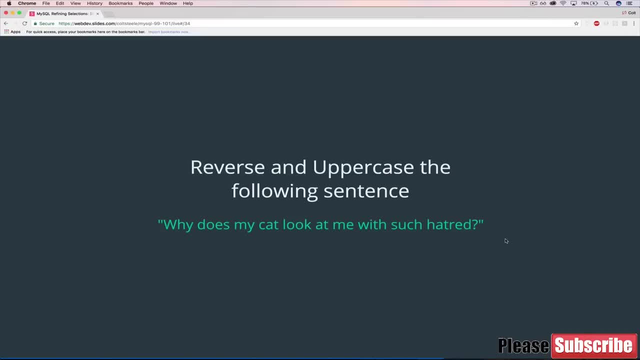 I should specify: don't just manually reverse it and type it uppercase. I mean using what you just learned. how can you reverse an uppercase this? All right. Then, when you're done with that, the next problem. this one's a little different. 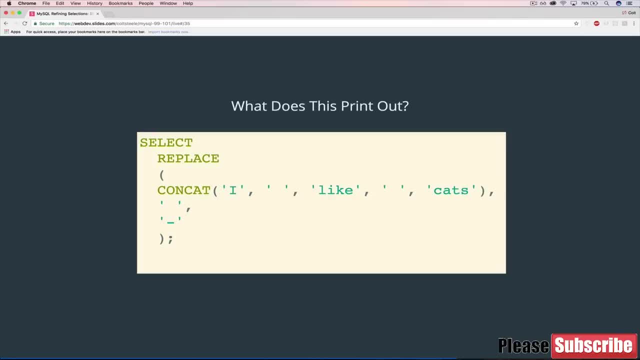 You don't have to actually do anything. I want you to figure out what this prints out, So don't just And copy and paste it. You can do that to check your work, of course. Uh, but try and work through what's actually happening. 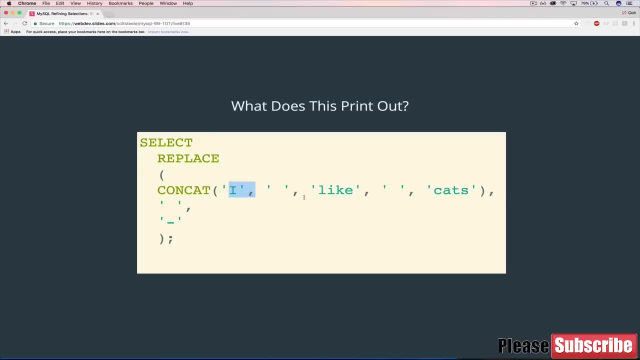 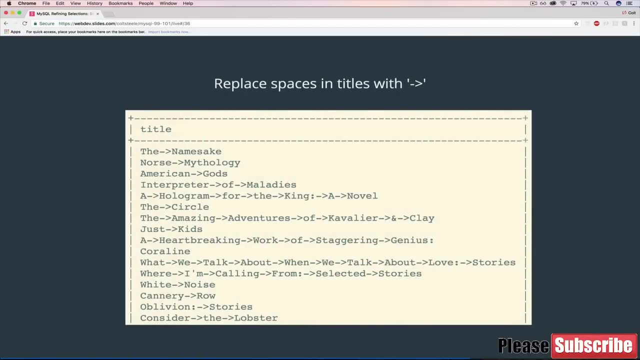 We've got to select, we've got to replace, and it can cat and some words and spaces and symbols and dashes. So we give it a shot. then move on to the next one here, which is to replace all the spaces in book titles with this little arrow. 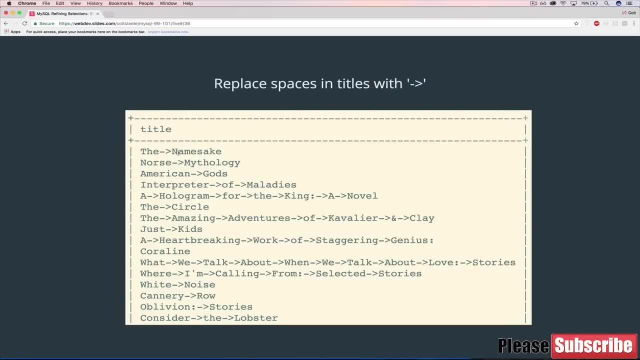 It's a dash greater than sign, So replace every space. So instead of the space namesake it's the Dash, or let's just say arrow, the arrow namesake. and that happens for every space. And one more thing I'll call attention to is up here: 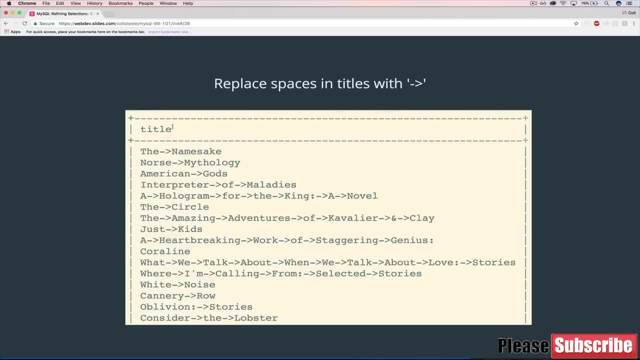 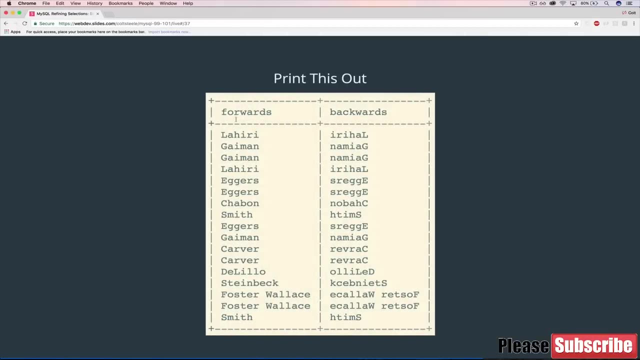 It just says title. So you're going to need to use as to make sure it says title. So, basically, your task is to just get this same data printed out, this exact same format, Then, after that, print this out, So you're going to have the author's last name. 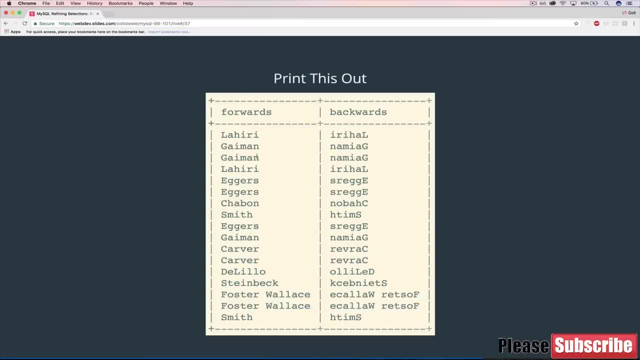 Printed regularly forwards, and then next to it you'll have the same author's name printed backwards in reverse. you might say so if that's what you need to do. um, also pay attention up here. it says forwards and backwards. 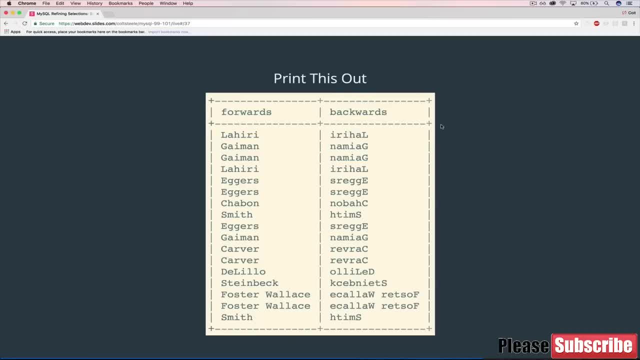 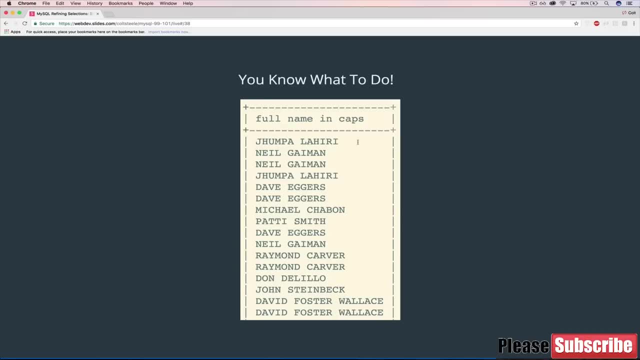 So you'll need to use as again to do that. Then, once you do that, the next one like you to print out a full author's name, So it's a little more complicated in caps. So we want Jhumpa Lahiri, so that's author first name and last name combined and uppercase, and that should happen for every author. 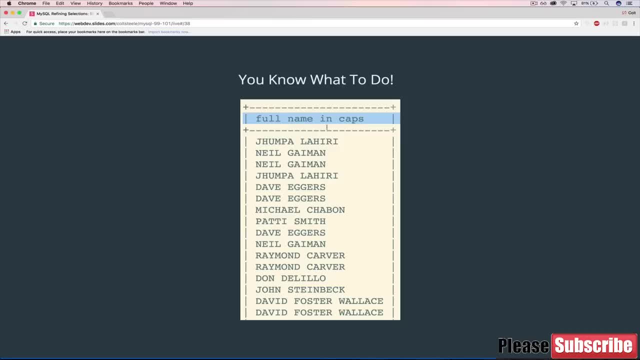 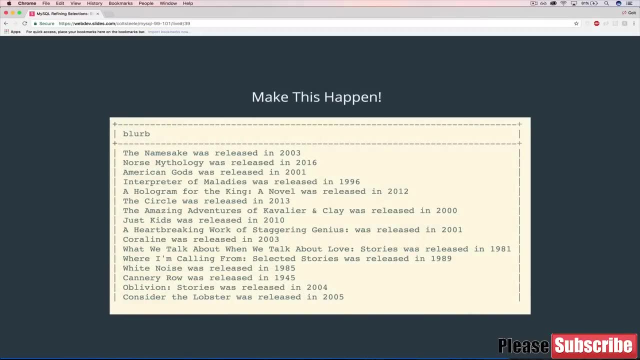 And then also again the name appears or the. the header says full name in caps. All right, then, make this happen. So what this is showing is a title, the namesake, and then was released in, and then the actual date that we have stored in our database for when it was. 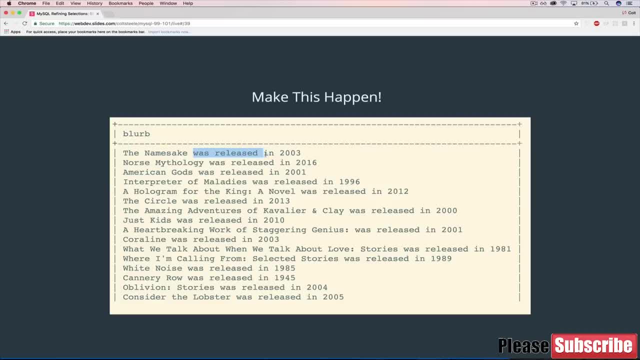 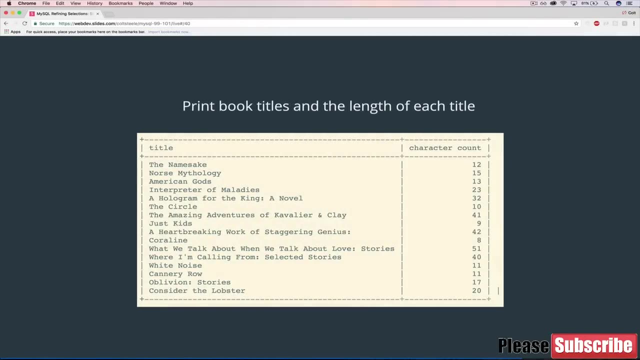 Released. So you need to combine a title was released in and then the year it was released. And again, I called it blurb, but just put some label up there. Then next one here print book titles and the length of each title, which is pretty similar to what I had. what I did, um, using author's last names. 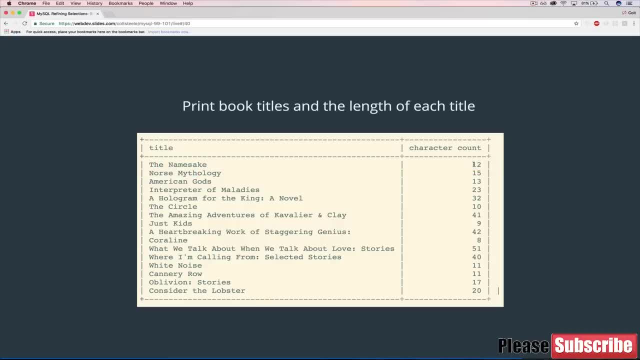 So just print the title and then the number of characters in that title. as you can see some of them are quite similar. So you can see some of them are quite similar. So you can see some of them are quite similar. So you can see some of them are quite similar. 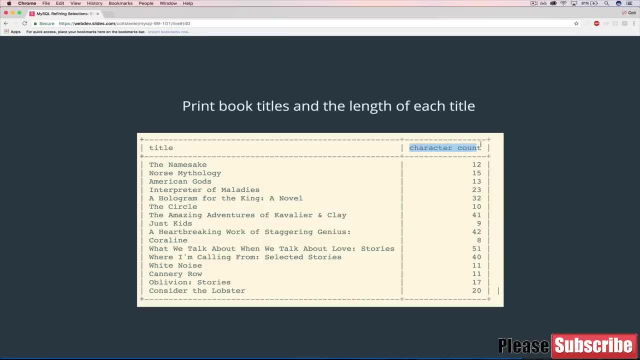 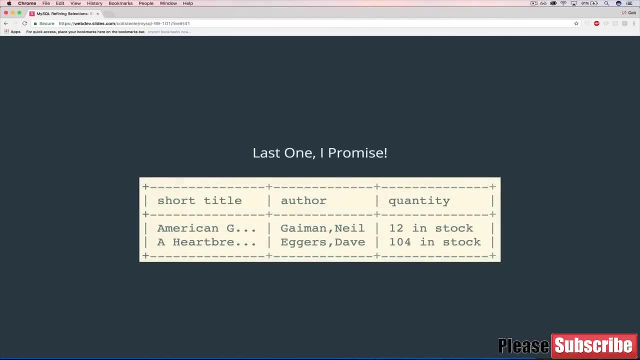 Uh, the only other thing I would say is: up here, pay attention, We have character count, So use as you get it by now. Then, finally, this one combines three different pieces of data. We'd like to have a shortened title. 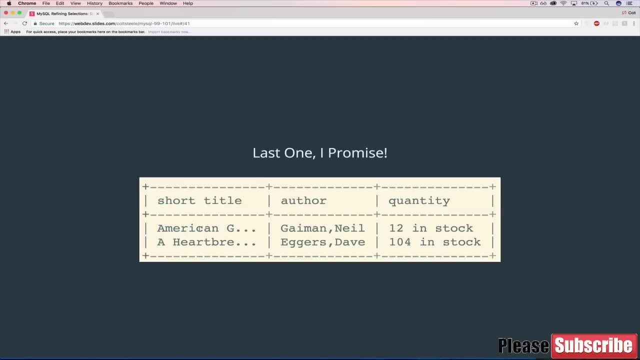 So I believe this is 10 characters: 1,, 2,, 3,, 4,, 5,, 6,, 7,, 8,, 9.. Yes, So the first 10 characters and then a dot dot dot afterwards and call that. 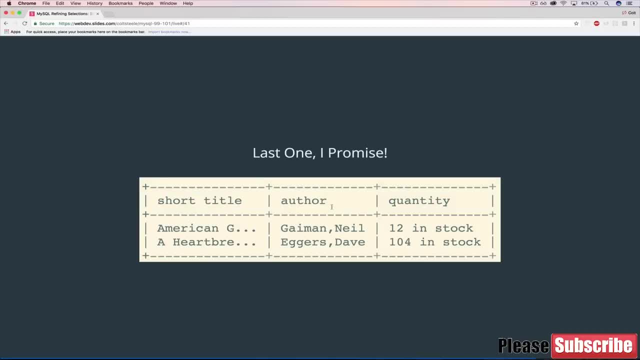 Short title, then we'll have the author printed out. but the way it should be printed is last name followed by a comma, followed by first name and then quantity. So quantity should not just be the number we have in stock, but it should be the sentence: 12 in stock or 104 in stock. 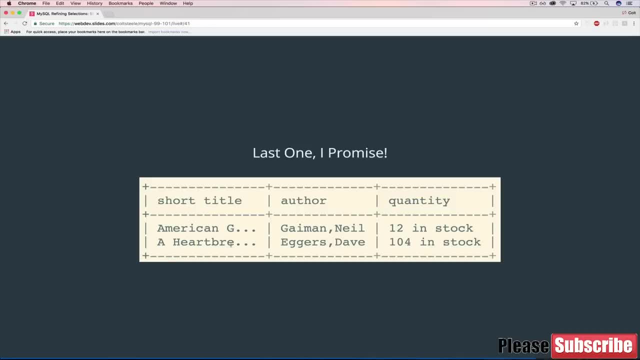 So there's a lot of pieces here, and each one of these three is going to require multiple string functions to make it work, So give it a shot. Um, this one is a little more challenging, so don't panic again if you don't get it. 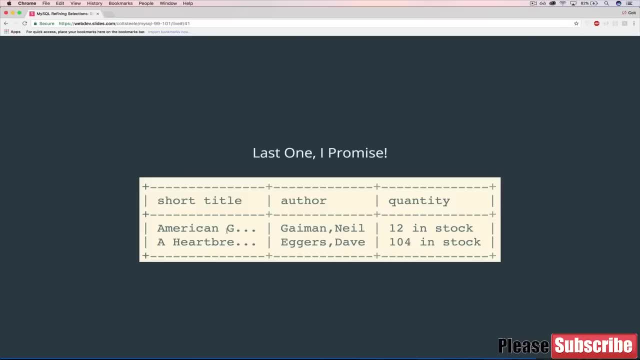 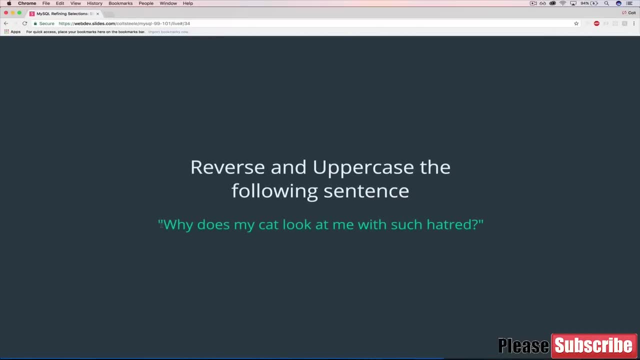 Uh, but try them all out, and then in the next video we'll have solutions. Okay, Let's go through some of these solutions. So the first one: reverse and uppercase this following sentence: Why does my cat look at me with such hatred? 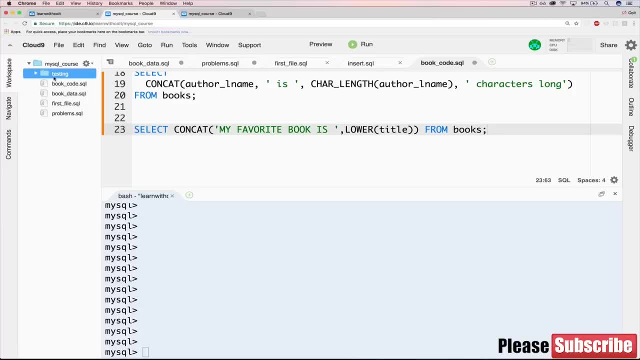 So I'm just going to copy it And the first thing I'm actually going to do is make a new file. So I'll come up here and do new File And I'll just call this exercises: dot, SQL. Then in there I'll paste this, and we know that we need to do two things. 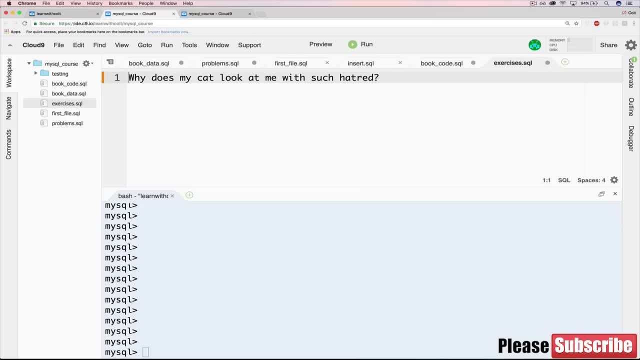 We need to reverse it in uppercase. The order doesn't really matter, So let's do a. we need to do a select first. either way, select, reverse, and we're going to select the reverse of this, and then we can do upper here. 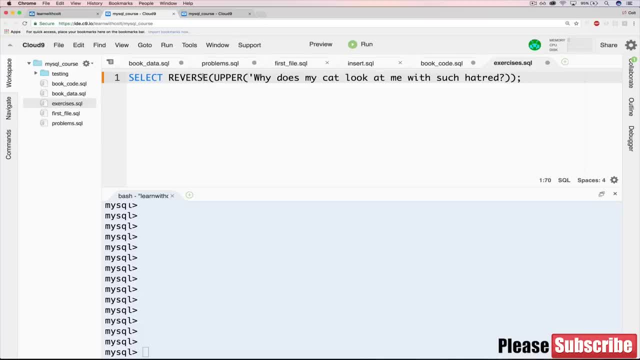 Just like that. Or we could switch them and do select upper, reverse. but let's give it a shot And I'm missing my quote there. Let's get out of here Missing that closing quote. There we go, Try it again. 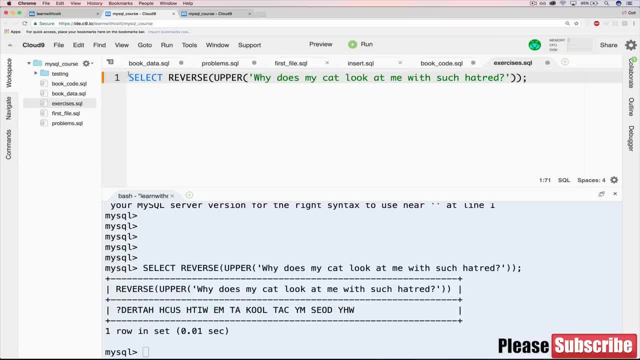 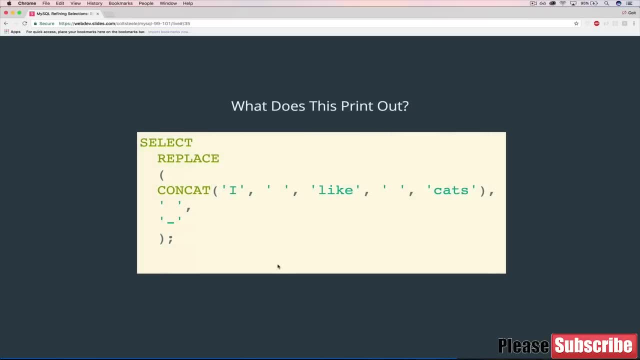 And there we go, It's reversed and all uppercase. So now I'm going to comment that out and we'll move on to the next one. What does this print out? So let's start on the inside. Concatenate I with space, with like space and cats. 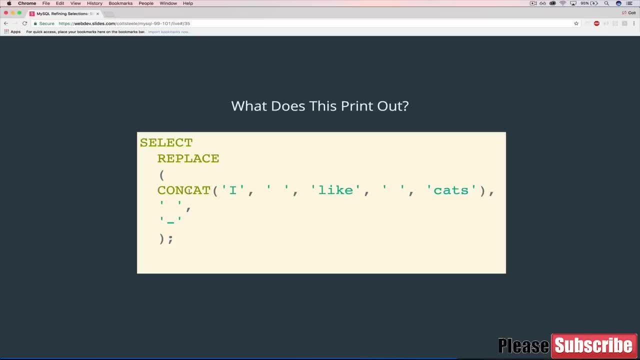 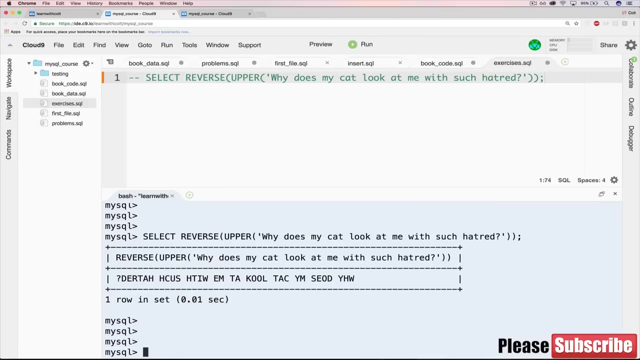 So it will be. I like cats, the sentence with spaces, But then we have a replace, and replace is going to get rid of all those spaces and put dashes. So it should be: I dash like dash cats. Let's try it. There we go. 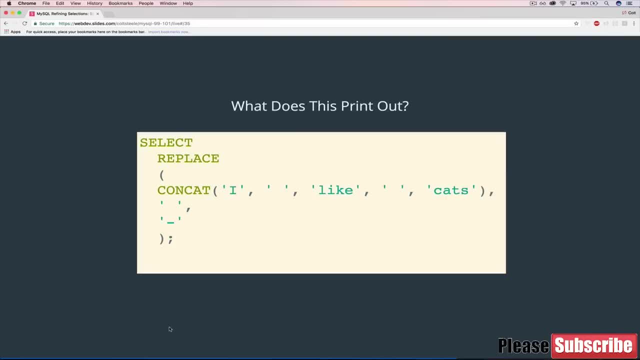 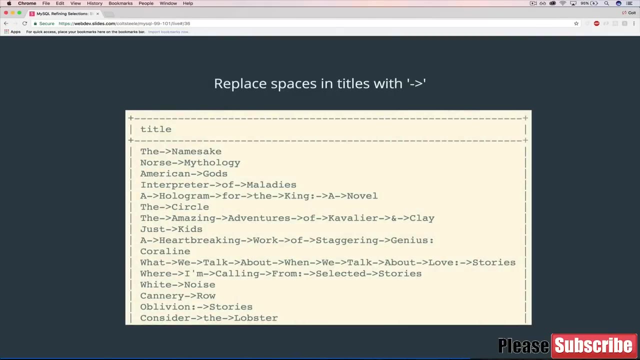 I like cats with dashes, So that one is really just testing that you understand how these are actually executed and that you can stack multiple or nest multiple functions. Next up we have our first one really working with the books data. So replace all spaces in book titles with the arrow. 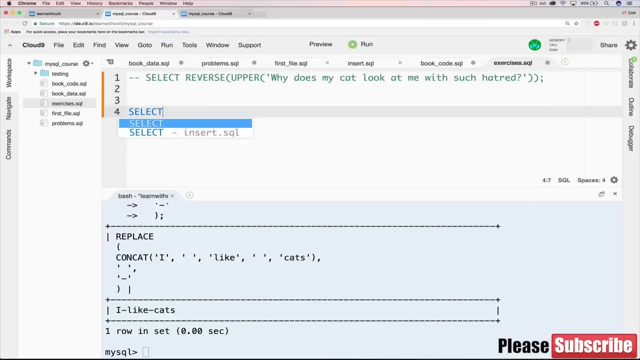 So we need to do a select and we know that there's going to be a replace And we know that it's going to be from books, So let's start with that. So what are we replacing? Well, we're looking for all titles and we're replacing a space with the arrow. 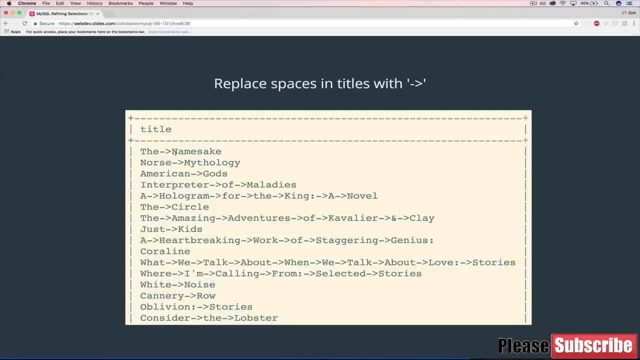 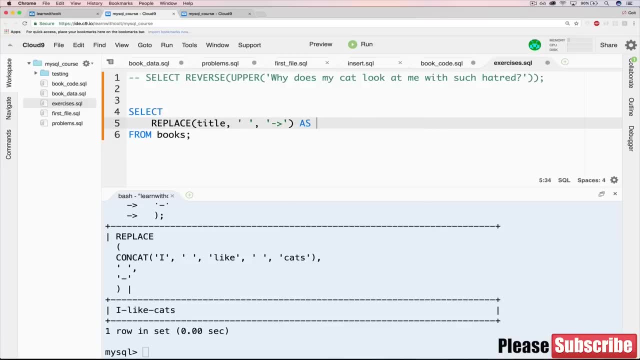 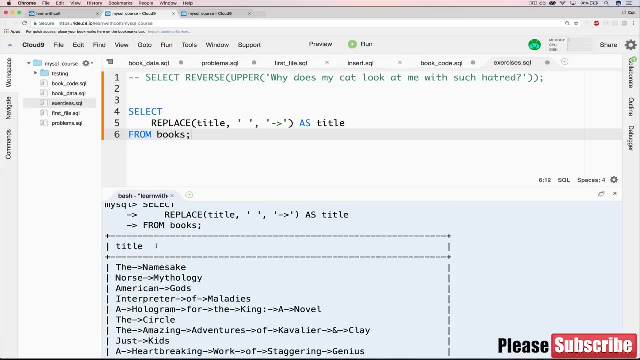 Double check, Replace spaces with arrows. That should be good. And the other thing was that up here we had title, So we need to use as title, So let's copy it. Make sure it works. There we go. Title: the arrow namesake, Norse arrow, mythology, and so on. 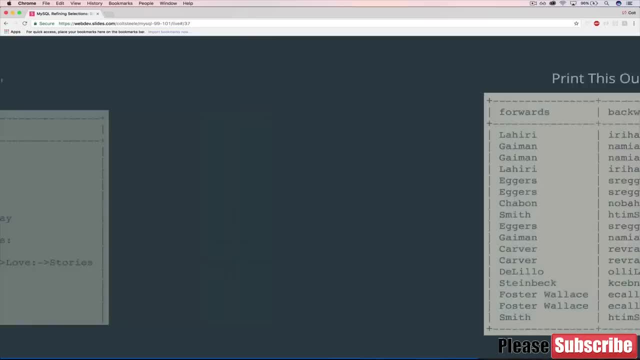 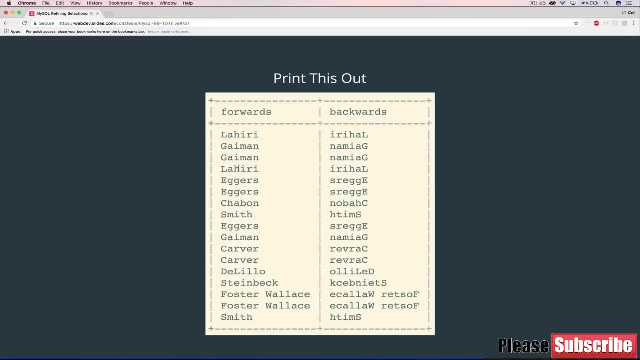 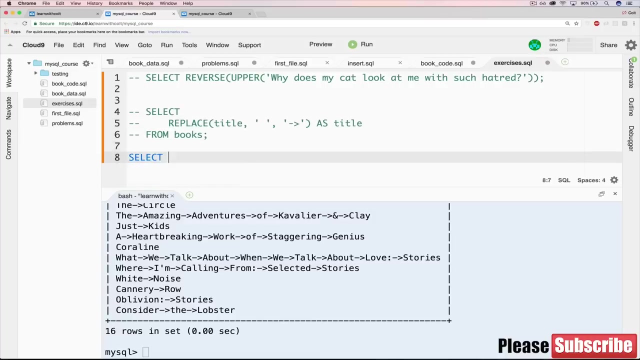 I'll comment that one out And we'll move on to the next one. Print this out: So we should have forwards and backwards- And this is last name printed regularly And this is last name reversed. So let's start. We know we need to have a select. 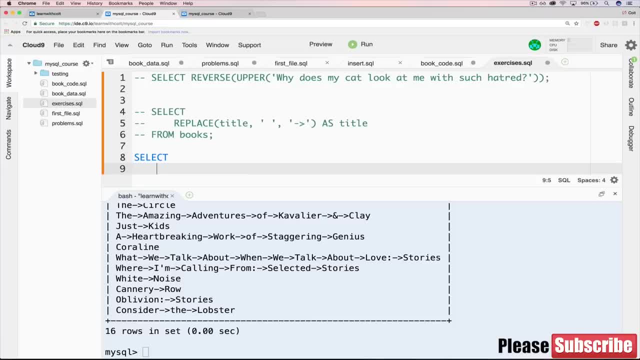 And the first thing That we know is that we're going to have author lname as forwards. Just make sure I have that, So that will give us this right here And let's close off. Let's do from books, Just like that. 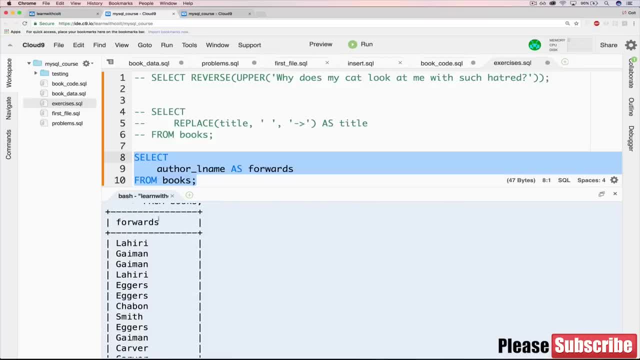 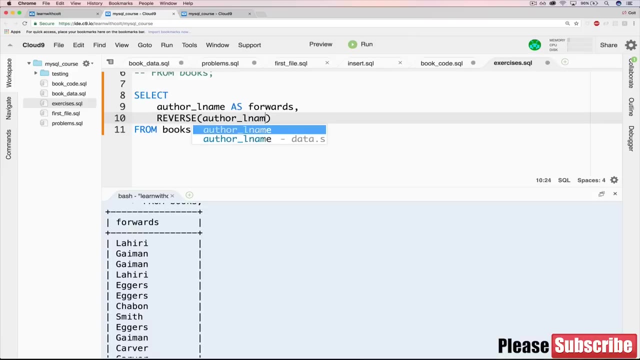 So we could start with this if we wanted, And we get that left portion. Now we need this right portion, So we need a comma, because we're now selecting two different things, And what we want to do here is use reverse author lname as backwards. 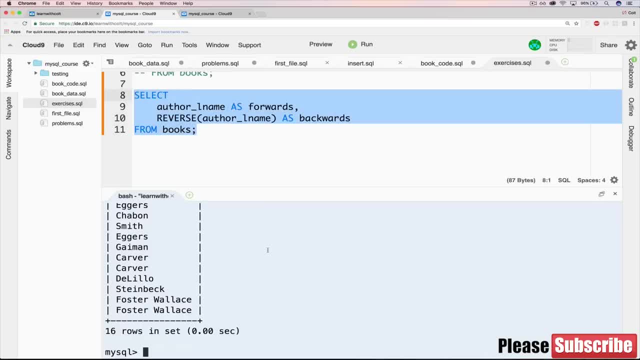 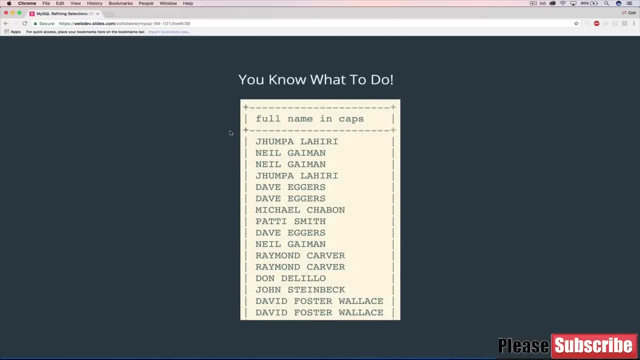 Just like that, Let's copy it And there we go, Forwards, backwards. regular last name, reversed last name. All right, Comment that one out And we move on This one. We need to print a full name. 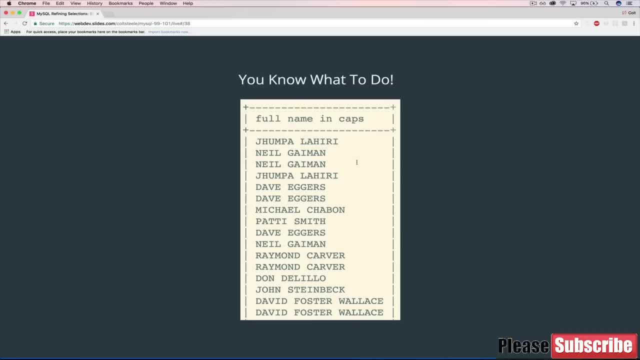 So first and last name of the author, all in caps, So there's a couple ways we could approach this. The easiest way is just to capitalize one string, So we combine the two, first and last, and then capitalize. If you wanted to, though, you could take capital first and then capital second. 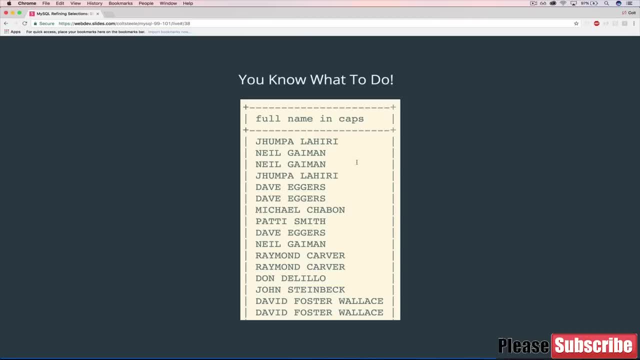 Excuse me, Capital first name, capital last name, then combine them And that works just as well, But it's easier to just do it once And it's also faster. So the other thing is we have full name- Full name- in caps up here, so we need to use as: 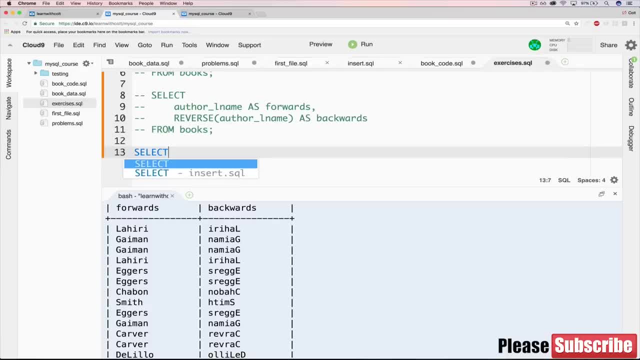 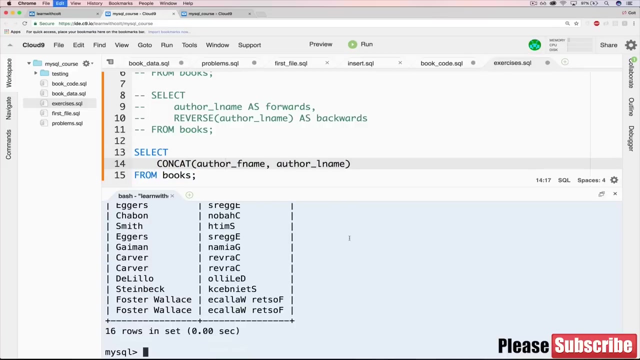 So let's start by printing full name. So we have a select from books And what we need to do is concat. And what are we concatting? Author fname, author lname, And I'll leave it like this for now, but hopefully you can predict what the problem is when I do that. 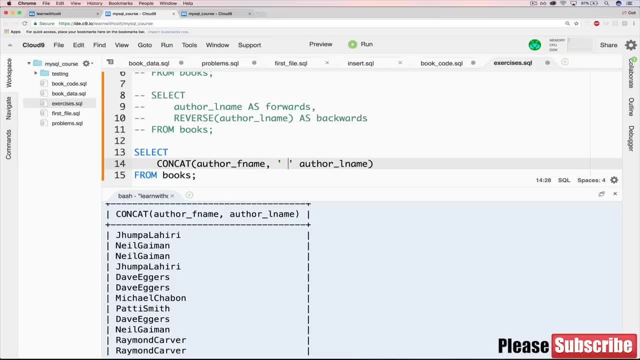 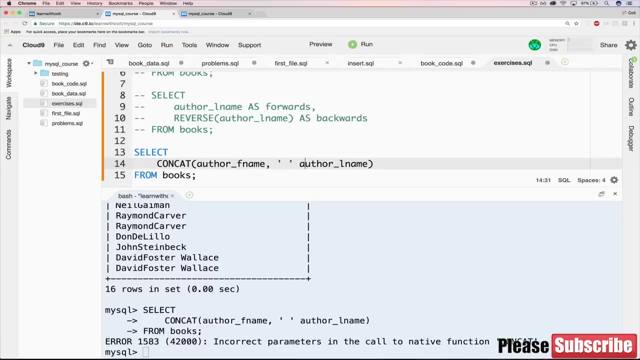 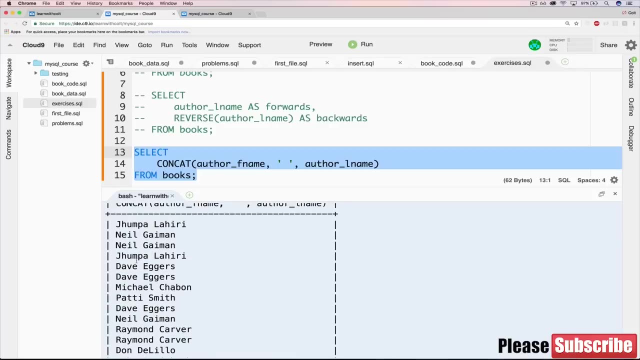 We don't have spaces, So let's add our space in, And that should give us the concatenated version. And well, if we add the right comma, Now let's try it. There we go. So we get Jhumpa Lahiri, Dave Eggers and so on, with the spaces. 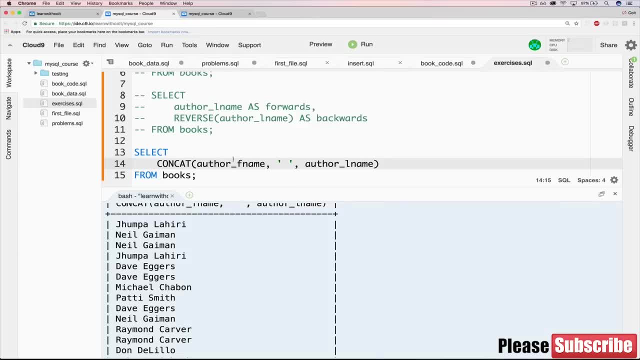 So now what we want to do is just uppercase that, So we could do it on the same line. because uppercase is so short, We can just say upper Above that, copy it, paste it in. We also need to rename this up there. 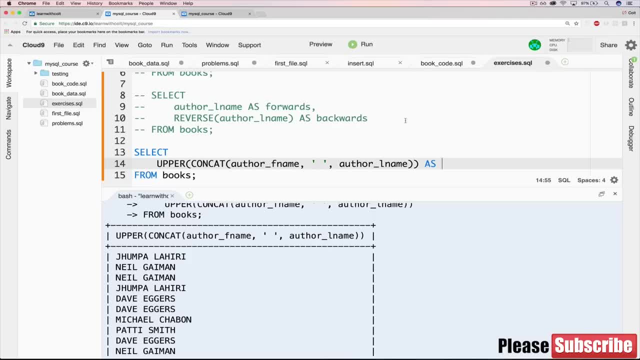 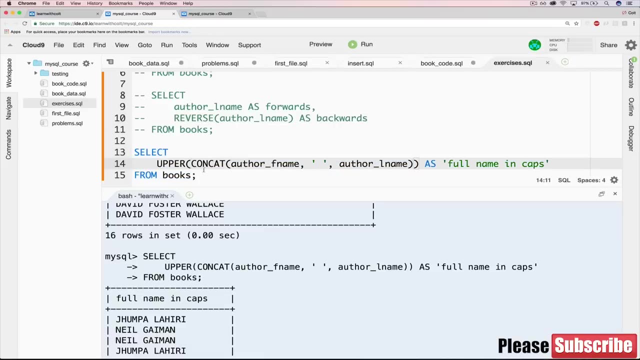 So we need as- and what did I call it? Full name in caps. So there's spaces in that, So we need to use quotes: Full name in caps. Copy that. There we go, Full name in caps. And if we wanted to format a little bit better here, we could do this. 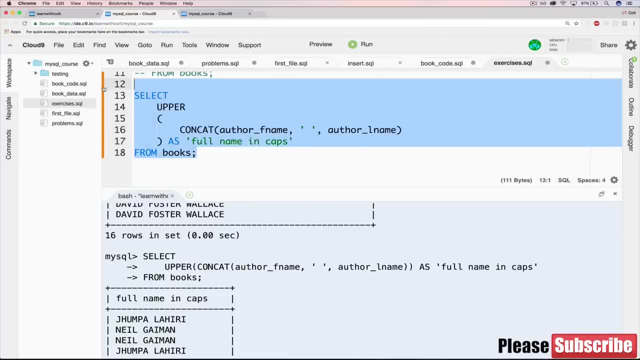 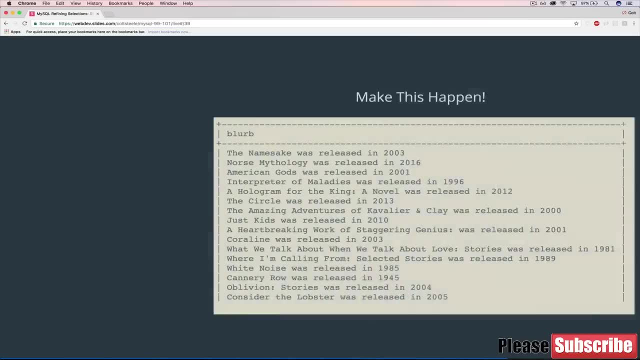 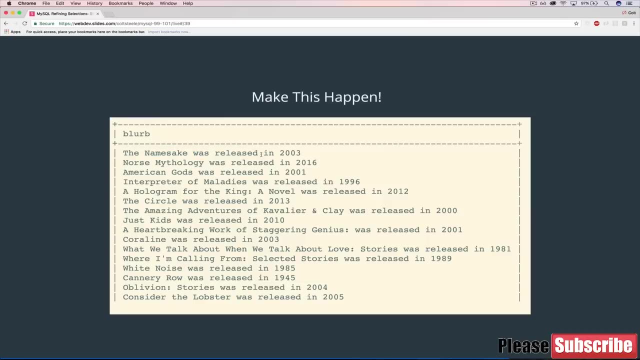 Just like that, And it will work just the same. Okay, Let's comment that one out and move on. Make this happen. So what we have again is the first- excuse me, the title was released in- and then the year, So we're going to need to make use of concatenate. 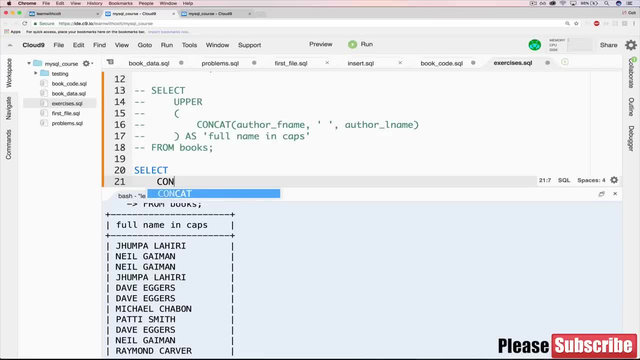 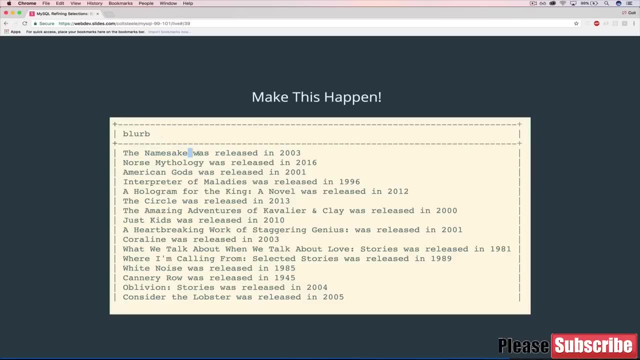 So let's start off with our select and we'll have a concat. Okay, So we will also have from books, just like everything else we've done. So what are we going to concatenate? Well, first is the title. After the title we have, space was released in space. 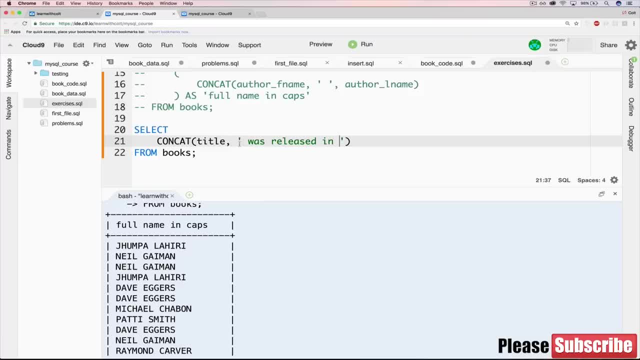 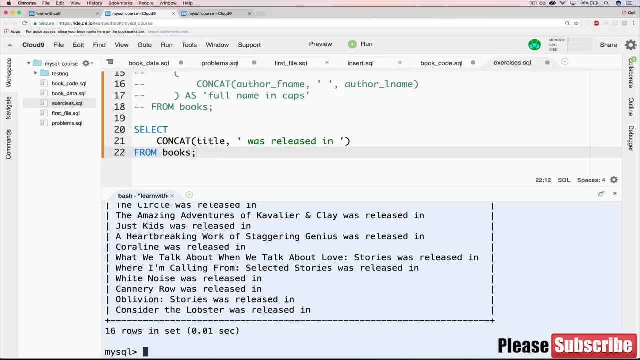 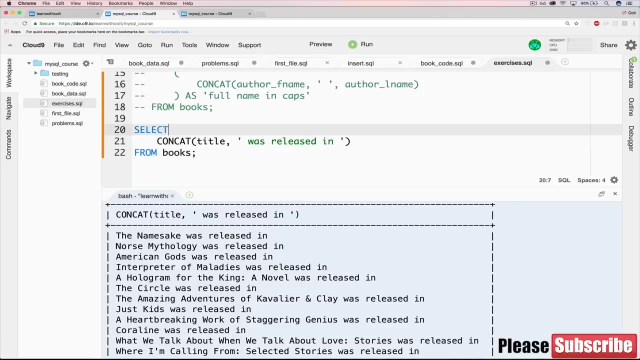 So we need those spaces comma like that And we could just start with that. if we want to take a look and we get the namesake was released in Norse mythology was released in, Okay, Then we just need to add in the year comma: released year. 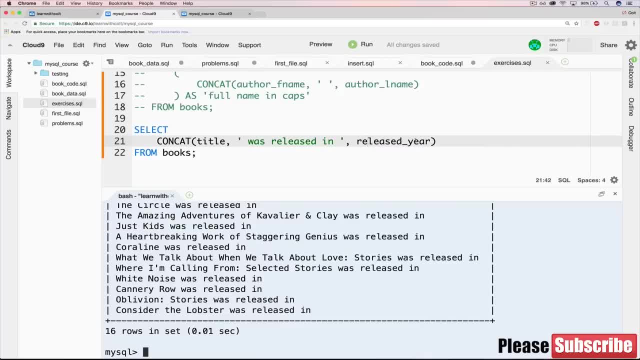 And we haven't really worked with the year in a while. So if you forgot what the name of that column is, earlier I, when I was recording something, I ended up having to redo it because I was referring to year rather than released year. 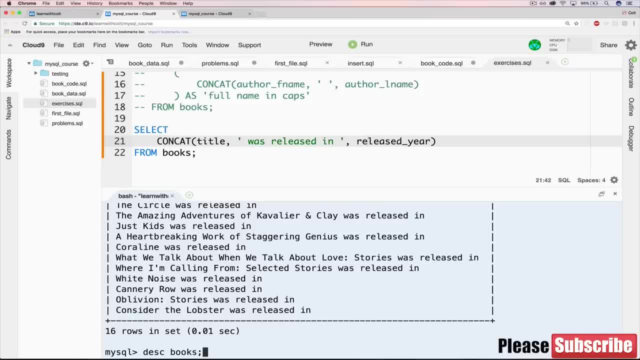 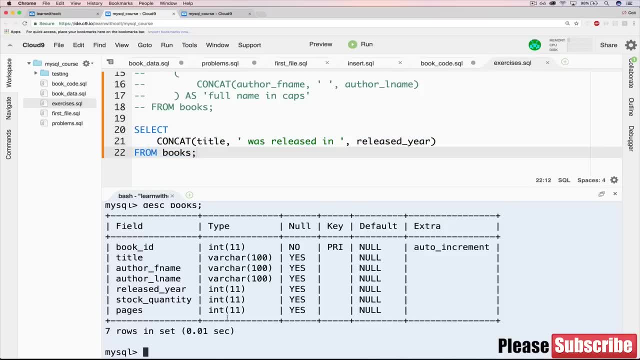 So you could just do a describe books and see that, okay, it's called released year. All right, So then we'll copy that in: Okay, Paste it and we get the namesake: was released in 2003, and so on. 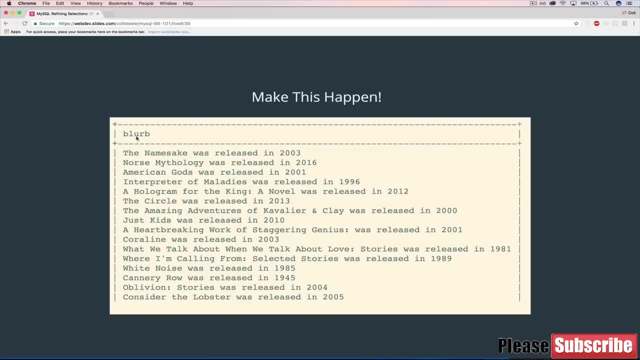 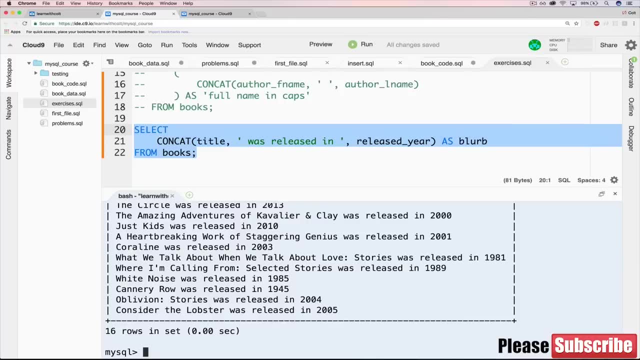 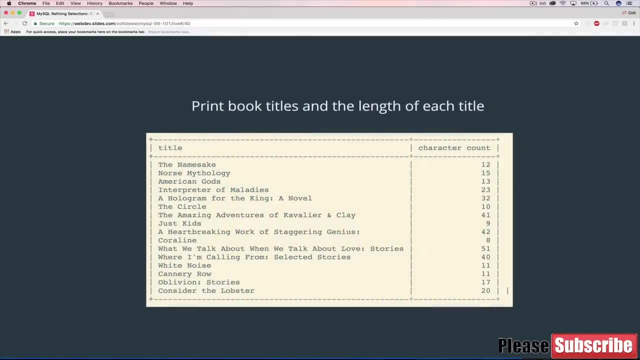 The only thing we need to change is this: up here It's supposed to be called blurb as blurb, And there we go, So we're done with that. one commented out Next up print book titles and the length of each title. 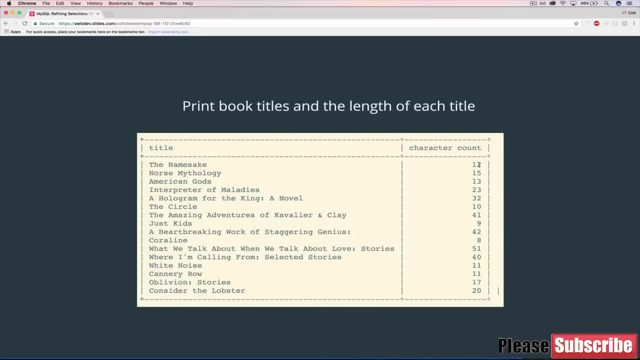 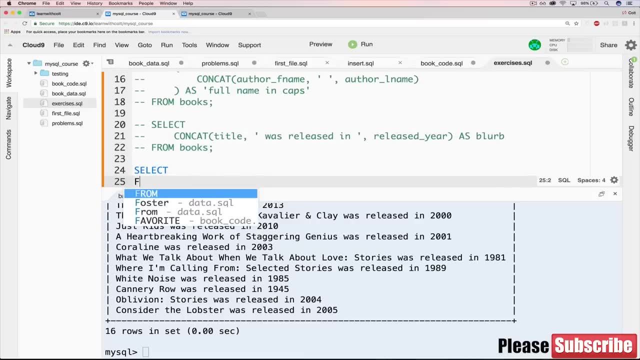 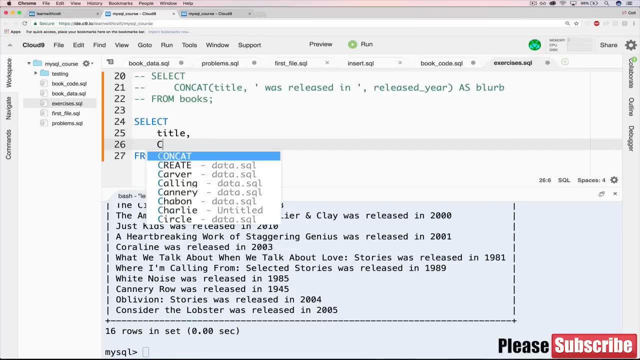 So printing the title is easy. Then we just need to use char length and print the character length. So let's do that now: Select from books. And what do we want to select? Well, first we want title And then, after we select the title, we want char length. 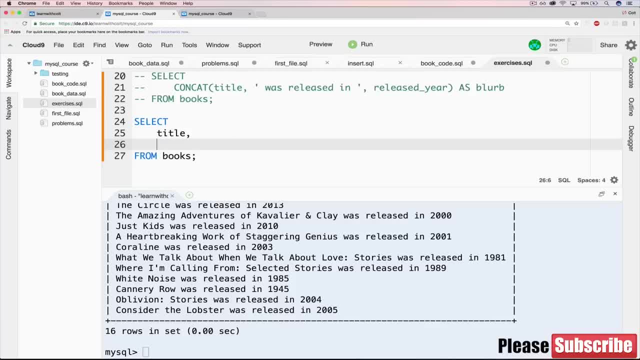 And one thing I should highlight there is that, because this is a SQL file, you might have noticed, I get these autocomplete suggestions, So I can either click or I can hit tab, And that's much faster. Okay, In my experience, is to hit tab. 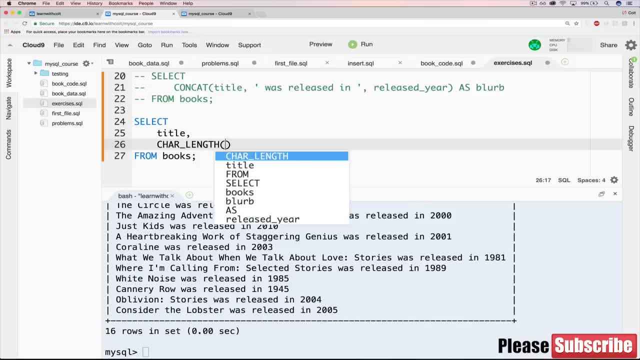 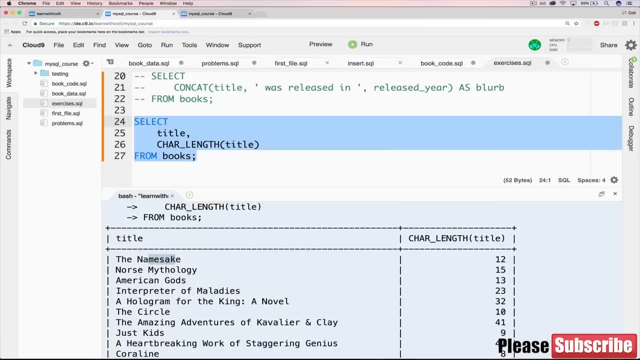 So we want the length of the title, Just like that, And we get the namesake 12, Norse mythology, 15, and that's what we want, except we need character count, Just like that. However, this will cause an error. whoops, we need to put it in quotes because there's 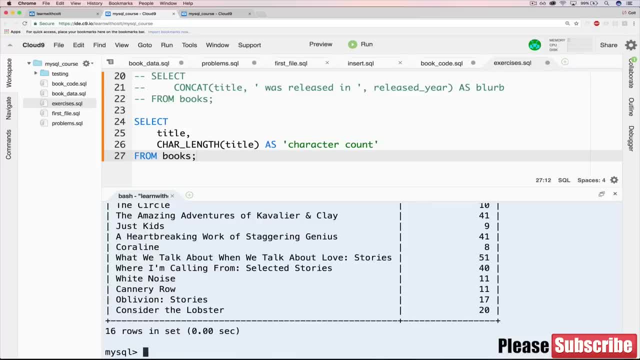 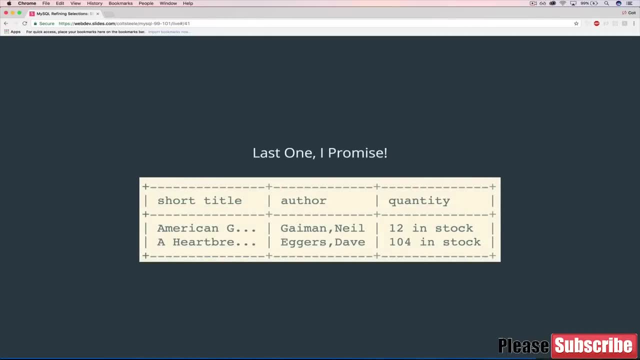 a space there. Now we give it a shot And it works Right. Last one, I promise. So this one is more complex. Three different things for selecting. Each one is complex on its own, So let's tackle the first bit, the short title. 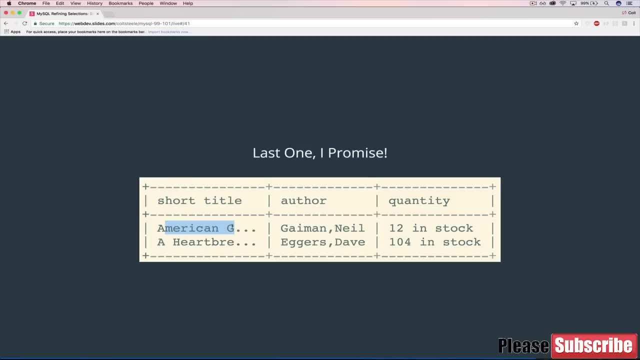 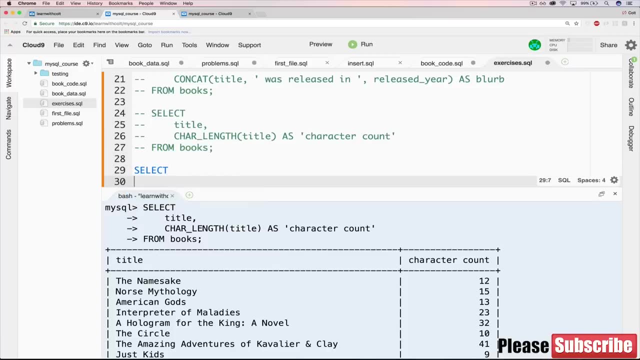 So we want first 10 characters of the title, plus dot, dot, dot. So we'll comment this out. We'll do our same, select from books And we'll start by selecting the first 10 characters. So that's substring. or if you're lazy, substr whatever, let's do substring. 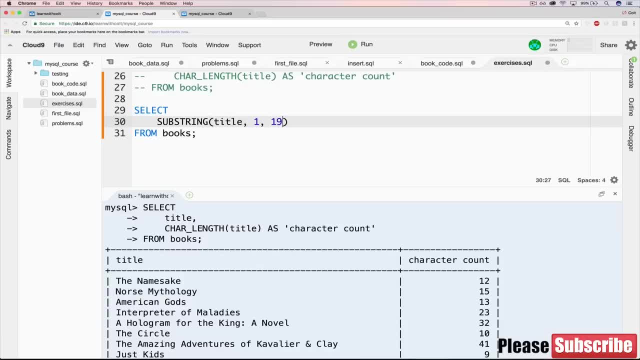 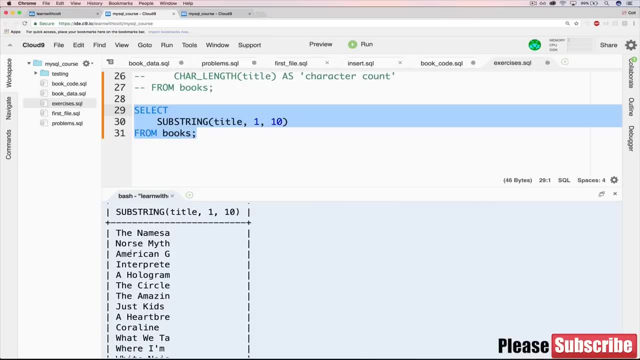 And we want it of title, from one to 10, just like that. So that should just give us at this point- you should know what it does- gives us the first 10 characters. But we also want to concatenate that with dot, dot, dot. 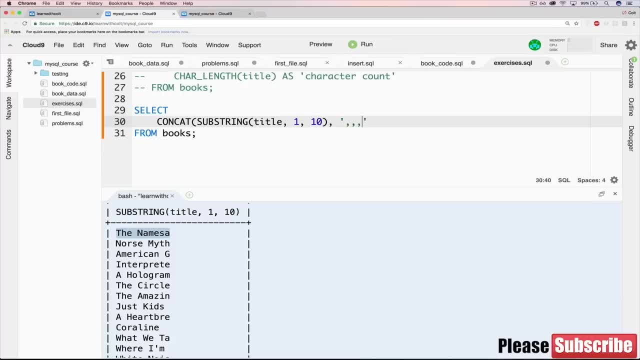 So we'll do that here, Concat, with the string dot dot dot, not comma, comma, comma, dot dot dot. And now if we copy that, that works, But it's supposed to be called short title, So we add as short title: 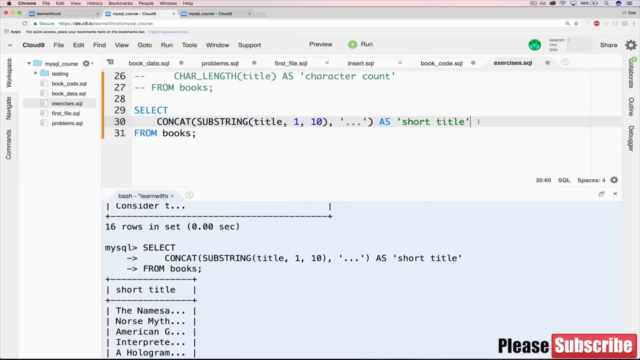 And we just triple check our work Looks good. Now we have our next thing. we're selecting which is the author, But we want last name comma, first name. So it's going to be another concat actually And we'll start with the author. L name comma- a comma in quotes kind of hard to talk about. 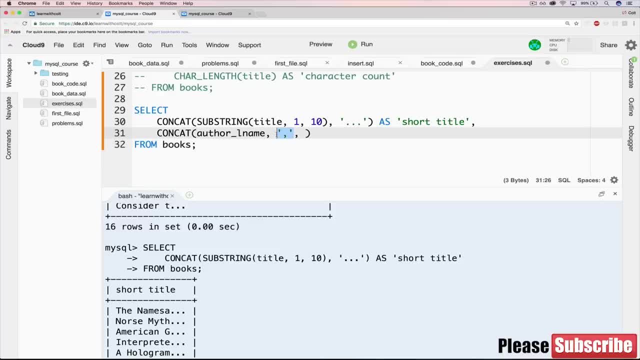 Comma, comma, comma. But this comma here is actually going to be concatenated in. This is quite easy. We've got a string to look at there- author F name, And we want it to be as author, So we don't have to use quotes for that. 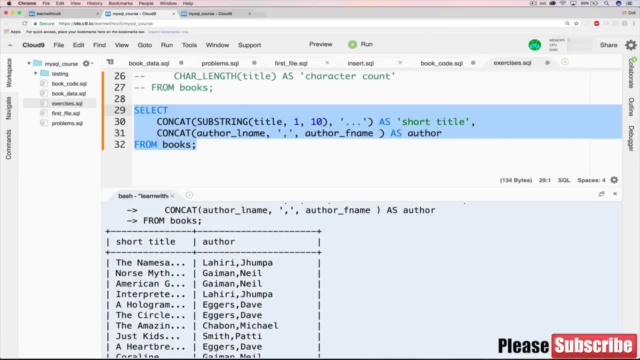 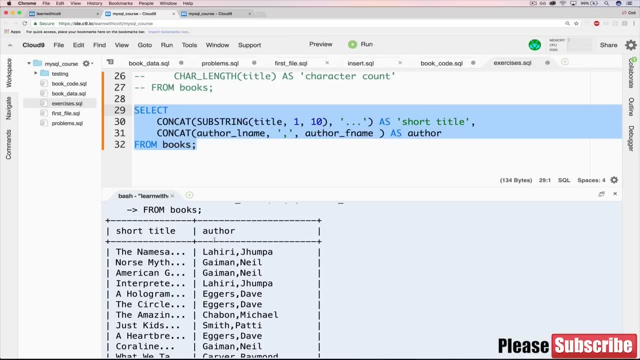 Let's try it, See if we made any mistakes. It looks good. So we get Lahiri comma Jhumpa, Gaiman comma Neil. That's what we expect, And it's called author Good. 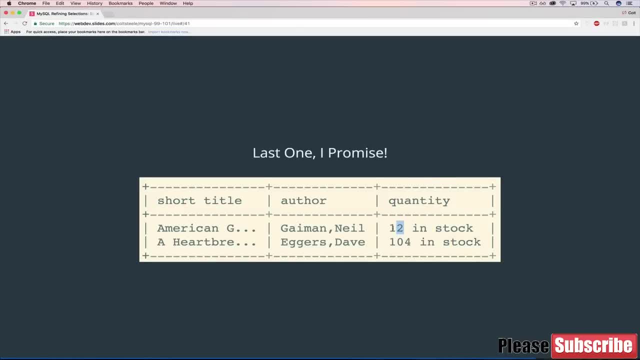 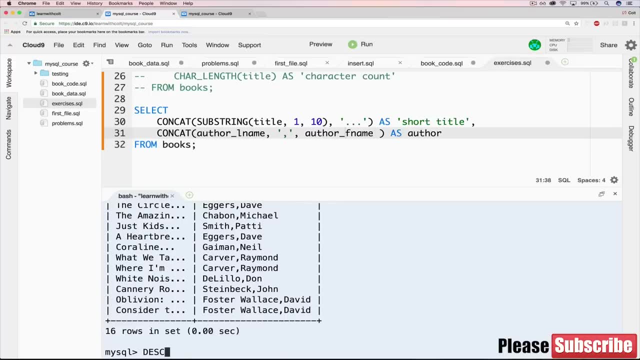 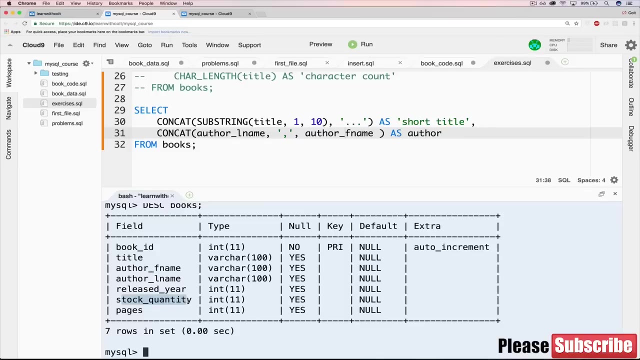 Finally, we need this last portion, quantity, And this should be the number in stock, Followed by the string in stock. So if you don't remember what the column name is, we can do describe books And you can see. OK, we have stock quantity. 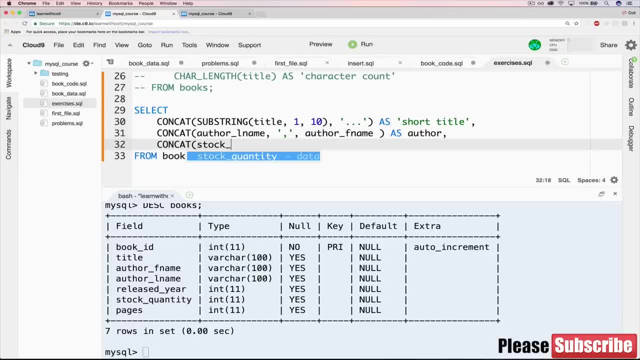 So that's what we want to use. So this time we're starting off with stock quantity comma, And then we want space in space, stock, Just like that- And then we need to use as quantity Boy- that's a long one. 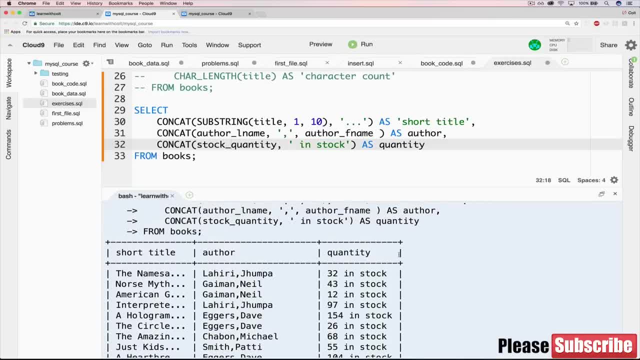 So let's try it out, Make sure we didn't do anything wrong And that looks good: 32 in stock, 154 in stock, And then we have author and short title both working. Now, one thing I want to point out here: 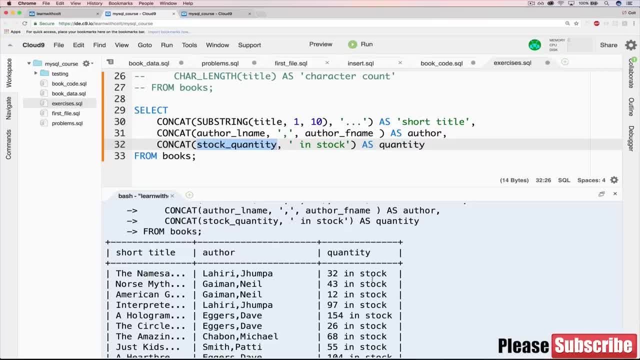 That stock quantity is a number, It's an int, But it doesn't break everything. Concat is OK with numbers like this. What it does is it just takes the string version- the text version- of 32, and adds it to in stock. 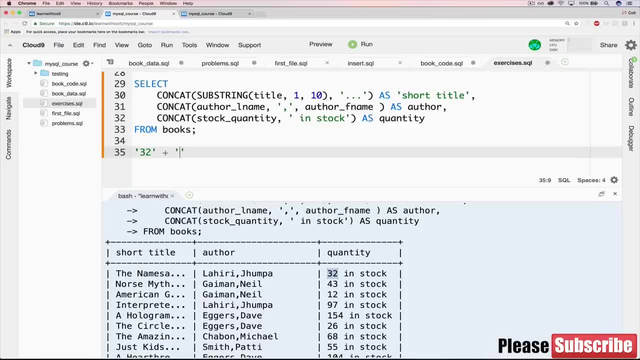 So it basically does this 32 plus in stock. So that's very different than trying to add a number to text. All right, So that was a lot, I know, But we're done now. We're done with these string functions. 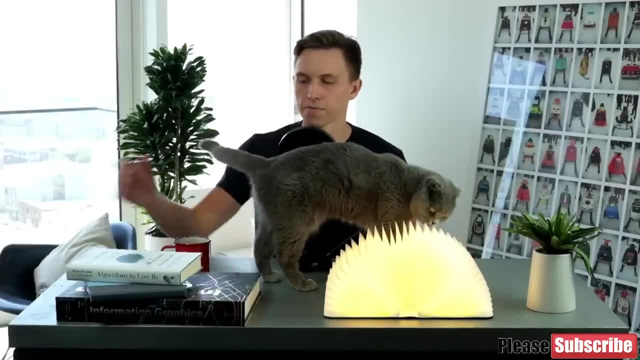 And we're moving on. Hey, welcome back. So this section, as you may have guessed, we're continuing on with our book stage And we're going to do a little bit more of that. We're going to focus on data. 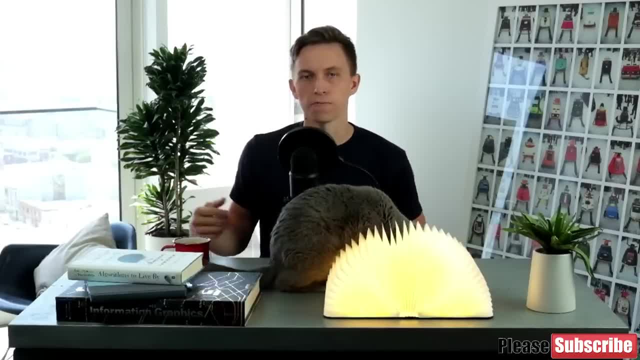 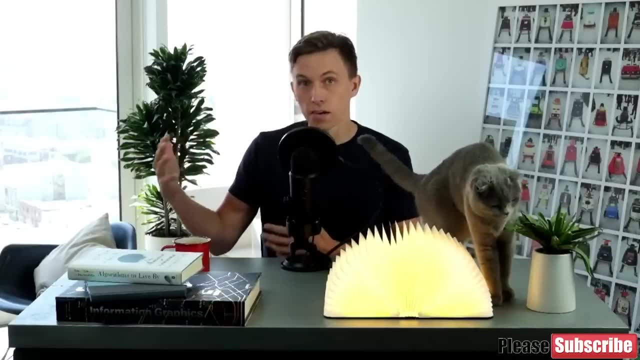 We're not doing cats, We're doing books, And primarily what we're going to do is focus on some more advanced MySQL features, things like limiting the number of results that we get back Instead of 10,000,. I want five. 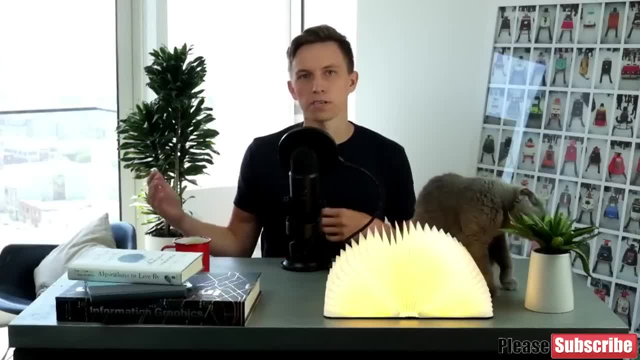 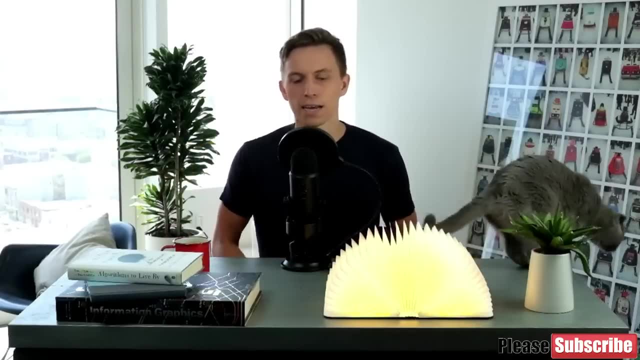 Then we'll see how to do things like sorting our results. I want the top five books sorted by sales, or sorted by title, alphabetically, or by genre- all sorts of things we can do- And then from there, of course, at the end we're going to have some fun exercises and 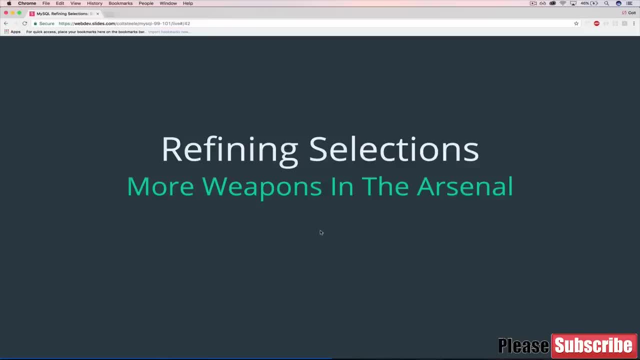 challenges to wrap everything up. So let's get started. All right, Welcome back. So in the last couple of sections we focused on select, And we're going to continue that trend. In this section, we're going to talk about some of the other tools that we'll be able. 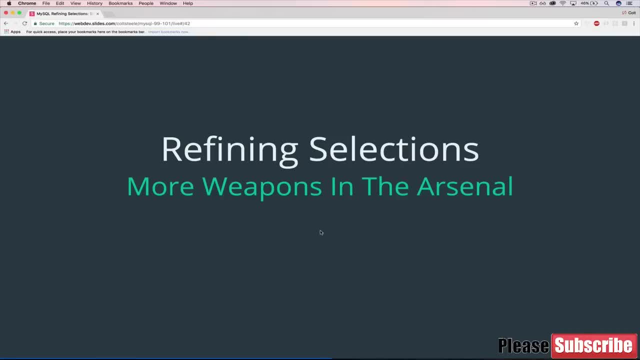 to use, to get more specific when we're selecting things. So we'll be able to do things like sort our results that we get back in alphabetical order or reverse alphabetical order or limit the number that we get or only get unique results back, and a bunch of other things that we'll be able to combine and use just as other tools. 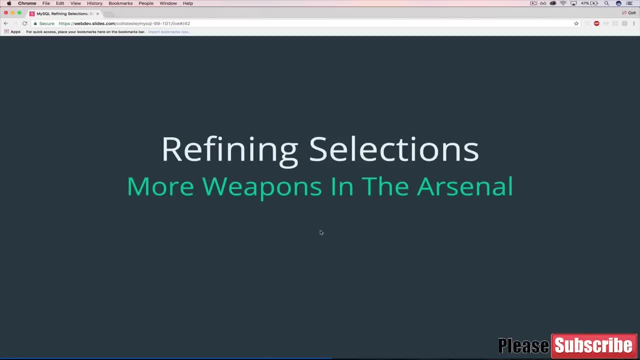 In our arsenal, or weapons, rather, in our arsenal. So before we do that, though, I want to start by just adding a little bit more data to the books that we're currently working with. Basically, I want to have a bit more variety. 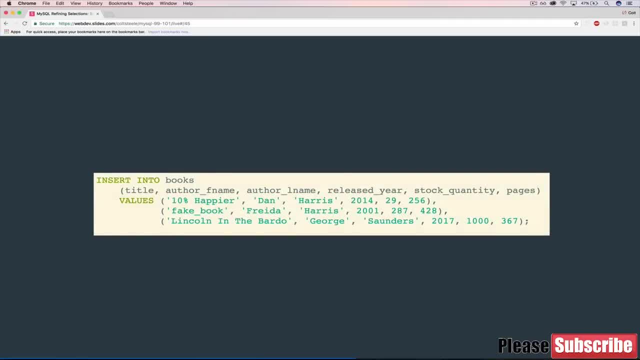 So I'd like to insert three new books, and they look like this. So we have one here: 10% Happier, by Dan Harris, released in 2014.. We have 29 in stock and it's 256 pages long. You'll see why we have that, why we're inserting that, in just a couple of videos. 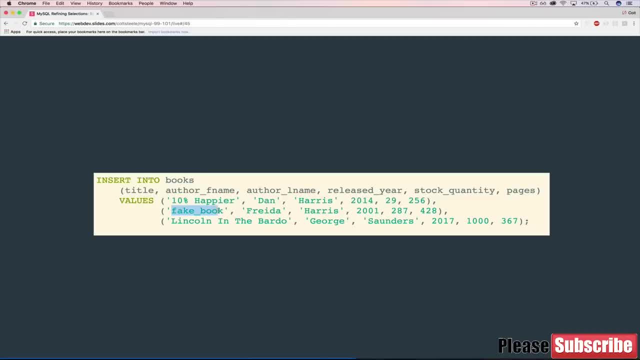 But there is a reason, we're going to come back to it. And then we have a fake book. So just imagine that we're testing our system or something and we want to make sure it works, So we have fake underscore book. And then that's written by Frida Harris in 2001,. 287 copies in stock, 428 pages. And then this is actually one, So I haven't read either of these, but this is one I just finished And that's one of the reasons I added it in. There's another one, though. It's really good, by the way, if you're looking for a book called Lincoln and the Bardo by 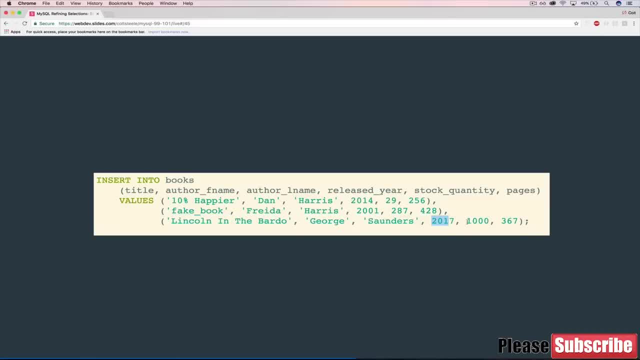 George Saunders released just this year And we have a thousand copies in stock because it's brand new. So we haven't sold any, or we haven't sold many yet, or maybe we're anticipating a big flood of sales. and it's 367 pages. 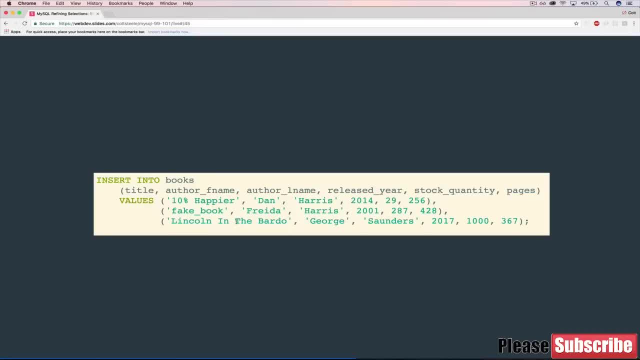 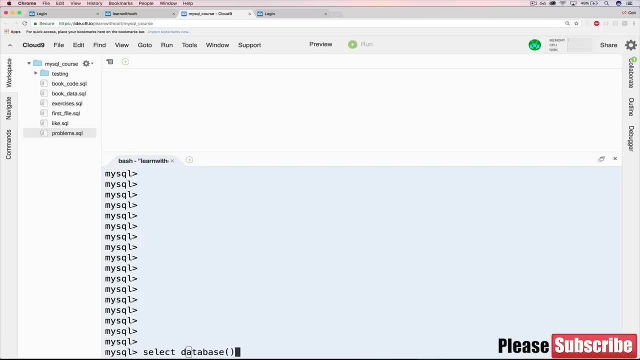 So either type that up or copy and paste it in the codes available along with this video. We're going to just copy and run over here. make sure that we're doing. let's make sure we're working with the correct database, All right. 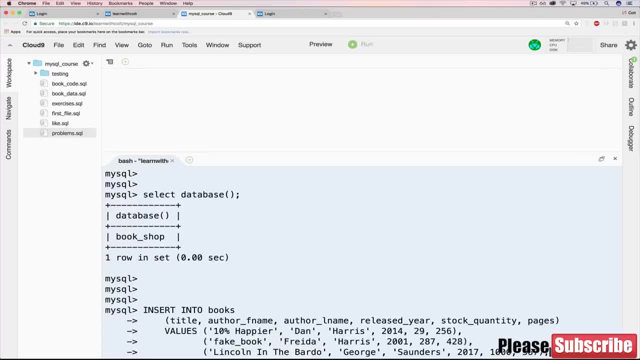 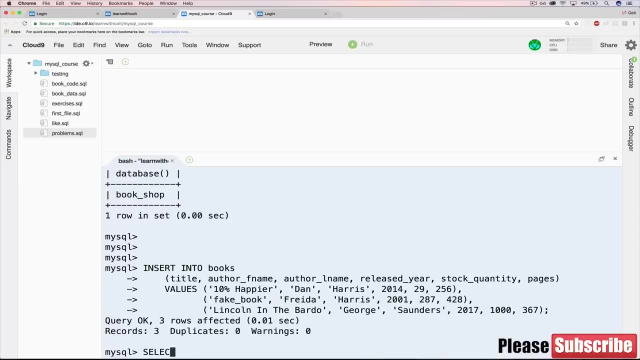 And bookshop And we'll just paste that in insert into books. blah, blah, blah, blah blah. We don't need to go over everything, All right, So we get three rows affected. Let's do a select title from books. 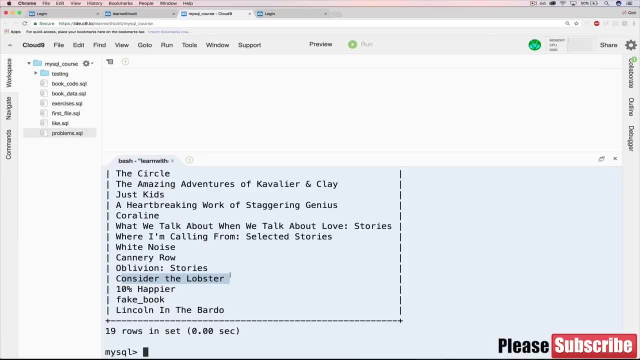 Just make sure that we have those in there. Here we go. We had up to consider the lobster in the last section. Now we have 10% happier fake book and Lincoln and the Bardo All right. So that's all I wanted to do here. 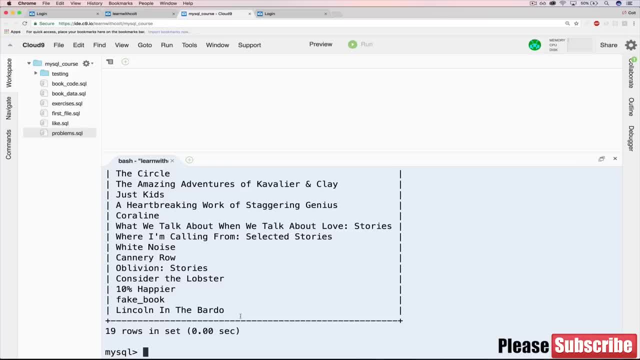 I highly recommend that you go and do this If you want to follow along. it will make the exercises much easier, It will make them possible in the first place And you'll be able to type the code that I type on your own. 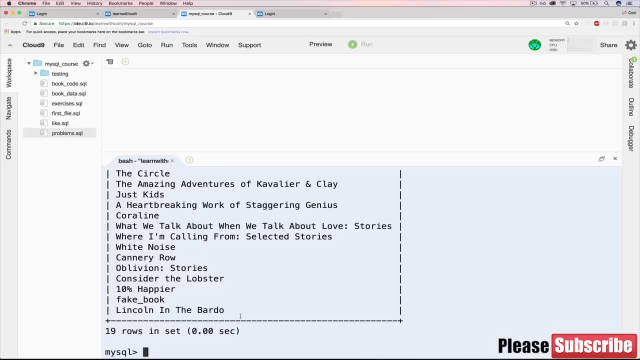 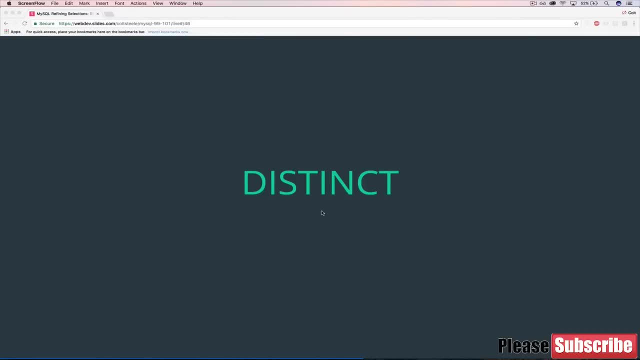 So I highly recommend that you do it, But I guess you could just watch if you wanted to. So, without further ado, let's get onto the new stuff. Now then I don't really like now then I use all right too much. 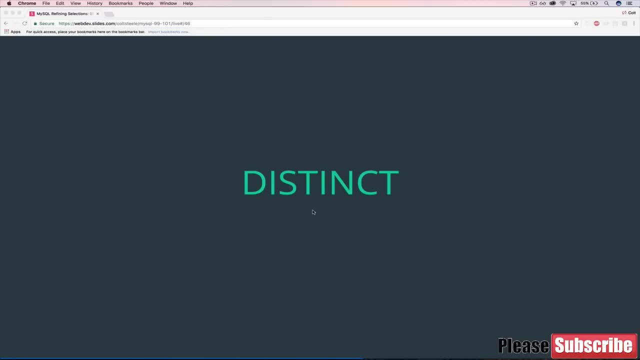 Okay, How about up? next, We're going to talk about distinction. We're going to talk about distinct. So distinct is something that we use in conjunction with select. So when we're selecting data out, let's say we're doing something like give me all book. 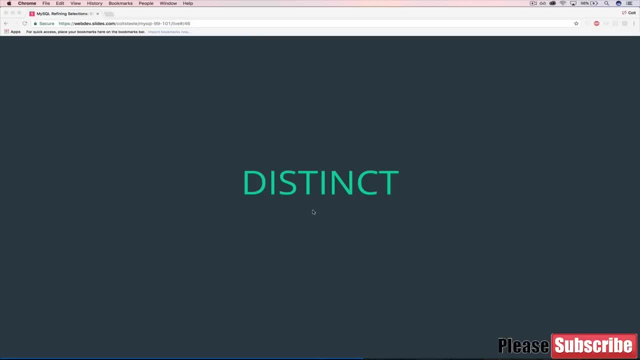 titles from the database and we may have duplicates in there and we would get all those duplicates because we just asked for all titles. But if I say give me all distinct titles, it will do what that sounds like. It will only give us the distinct or unique titles. 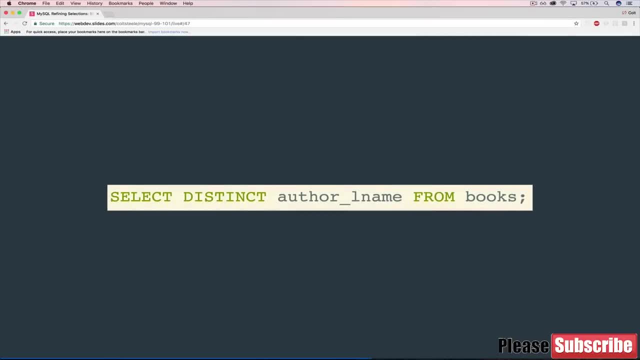 So, without further ado, let's take a look at it in use. So here's an example. The first thing that you should notice is that distinct comes right after select. So we're saying select author, last name. So there's a bunch of authors and in our table some books, have you know, or some authors. 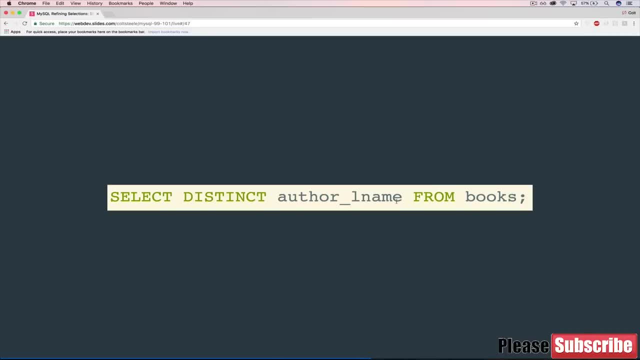 have multiple books. So David Foster Wallace, for example, has two books in there. So when we say select author last name, we get two results. We get David Foster Wallace and then again David. if we're only doing last name, we get 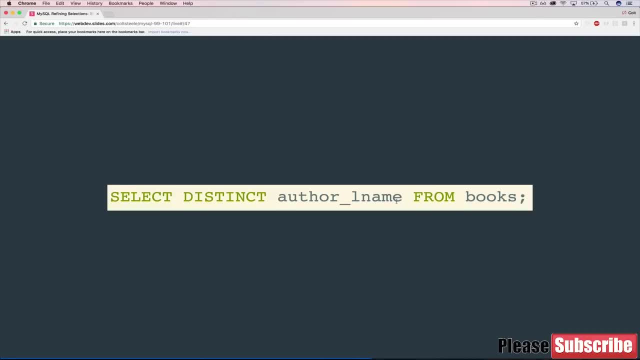 Foster Wallace and Foster Wallace. Okay, If I wanted to know only the unique or the distinct author last names in my books table, I would write this query here: select, And the only thing that's different is the distinct. So select distinct author name from books. 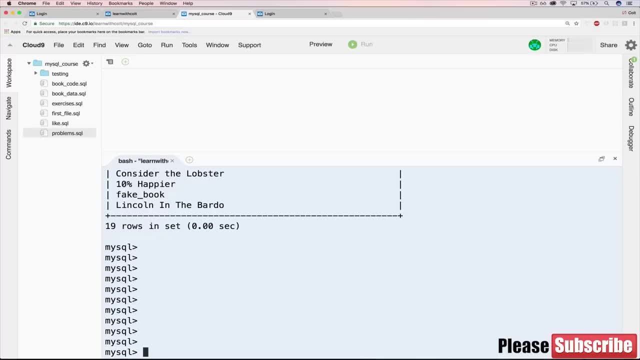 So let's try it out. We'll go over here, make some space and let's just start just to show you what I'm talking about by select author, without the distinct from books, Just like that, Okay, And as you can see, you know we have gay men. who's in here twice? 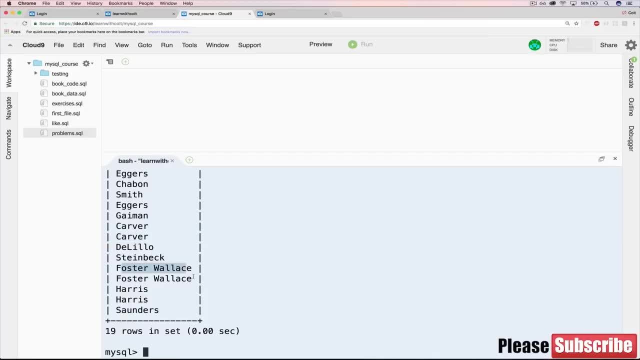 Eggers is in there twice, Carver is in there twice, Foster Wallace is in there twice and Harris is in there twice. However, there's something kind of weird about Harris that we'll take a look at in just a moment. Um so, if we only want to just get a survey of all the authors in our database, but we 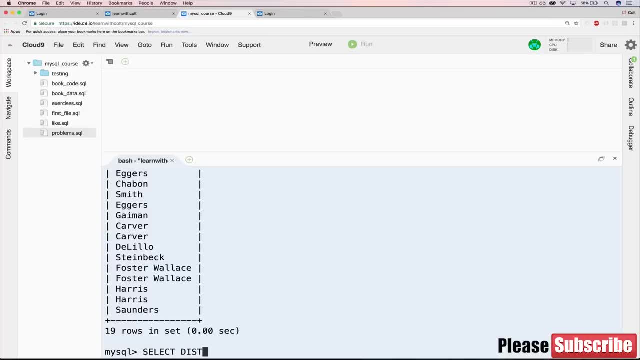 don't want duplicates. it's as simple as select distinct author L name from books, just like that. Hit enter. Now it's much shorter because those duplicates are gone. So now we only have one game and one Eggers, one Foster Wallace and one Harris. 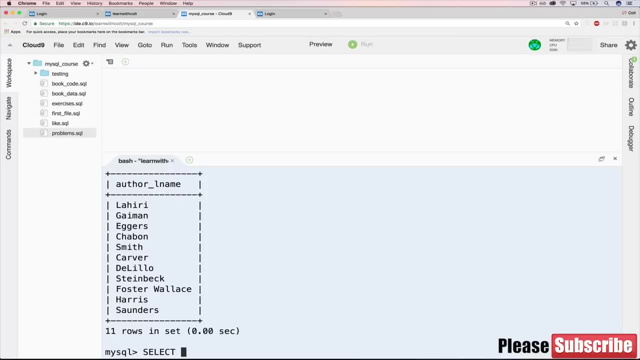 And of course we could do that for other things. So let's try it for years. So we have select released year from books. You can see. let's see are there some books that have duplicates? So, for example, 2003,. there's two 2003s at least. 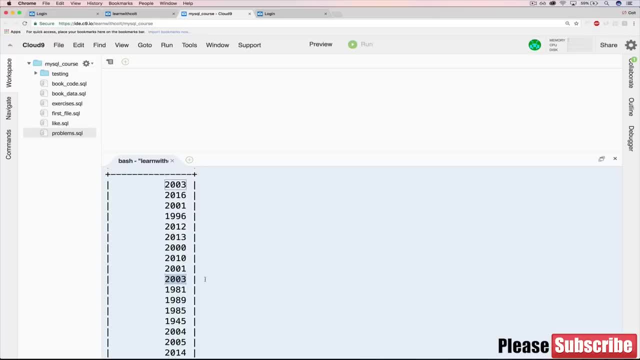 Uh, I think there's multiple. there's at least one more when I designed this or when I created the data. Let's just focus on 2003.. So there's two of them there. So if we do a select, distinct released year from books, our list is shorter. and now we 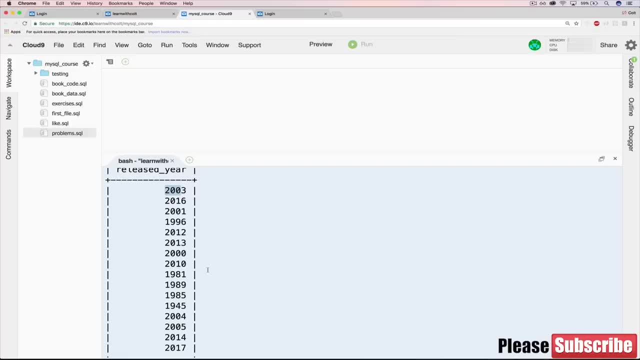 only have one: 2003.. So the reason I show it to you is not just to show you another way or another example, but also we're working with numbers here And that's important to remember that released year is an int, It's not a varchar, but distinct still works. 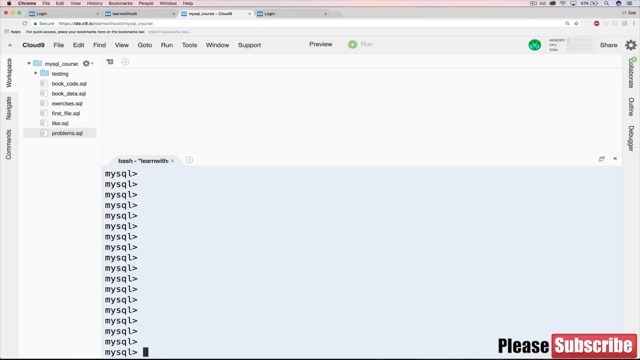 There's one more advanced thing that I want to talk about here, uh, which has to do with when we did our select- let's start again with author L name from books. When we did this, remember that there's, and actually let's do- author F name and L name. 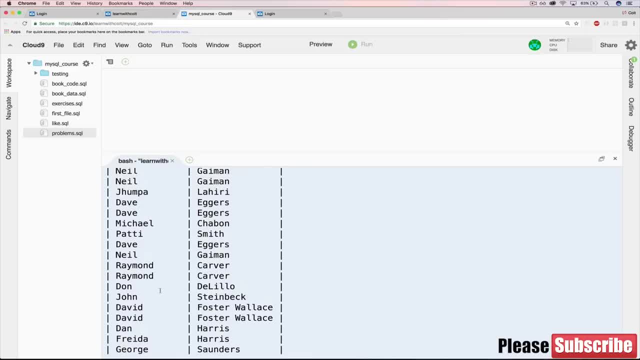 So when we did this, You know, remember, we have Neil Gaiman twice and Dave Eggers and so on, But then there was Dan Harris and Frida Harris: two different people, two different authors with the same last name, which is a pretty common situation. 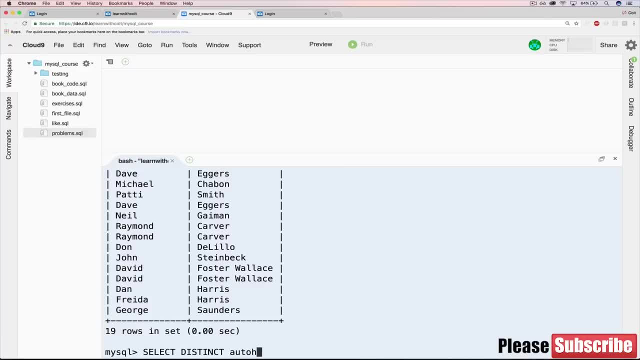 So when I do distinct, select, distinct author L name from books, it reduces them, you know, to just the distinct last name, which is what you would expect. It only gives us Once which makes sense. We're asking for distinct author last names, but what about distinct full names? 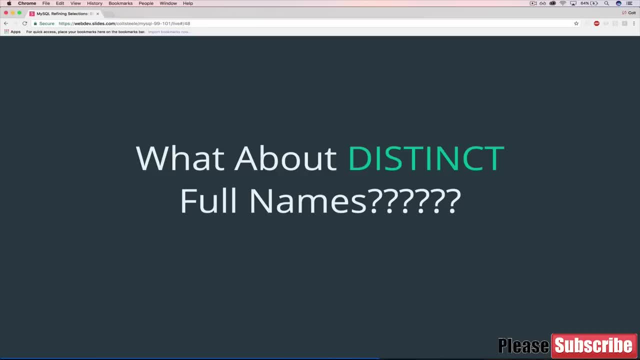 What if I want every distinct author's full name printed out? So, basically, what if I just want to know how many distinct authors there are, not just based off of last names or just first names, but both need to be distinct, so that you know. 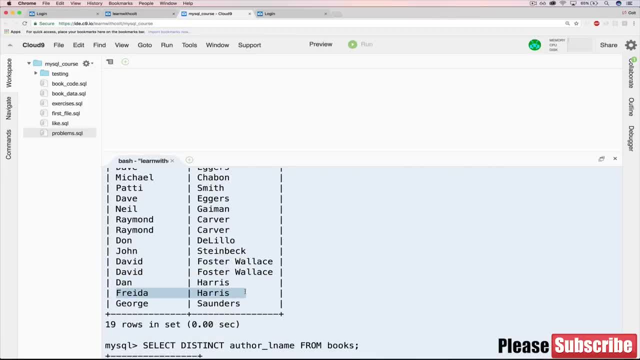 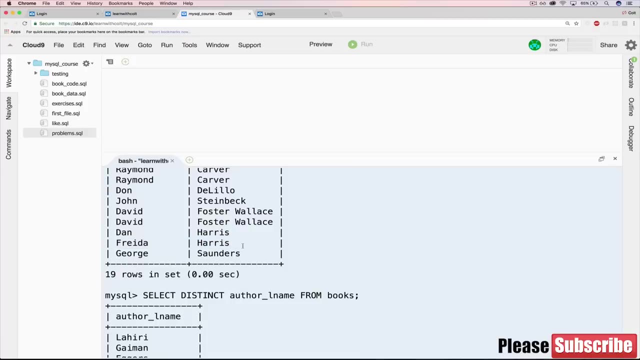 Dan Harris is distinct from Frida Harris. There are a couple of ways of doing it. One, If you already know at this point, you can use can cat, So I'll show you that Now. what we could do is can cat, author F name and author L name, and then ask or select. 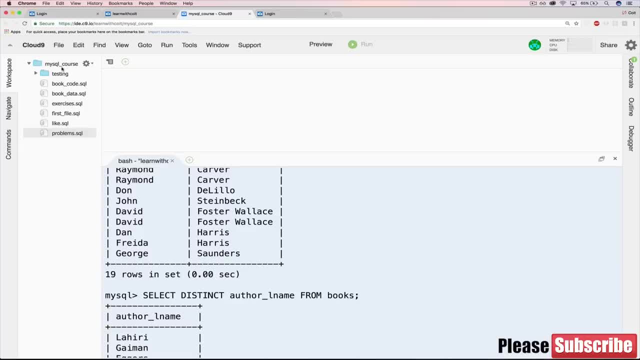 distinct versions of those. So if I make a new file, this one will be. it won't be too long, but I'll make a new directory first and I'll just call it refining selections. You don't have to do this, but I'm getting a little messy in here. 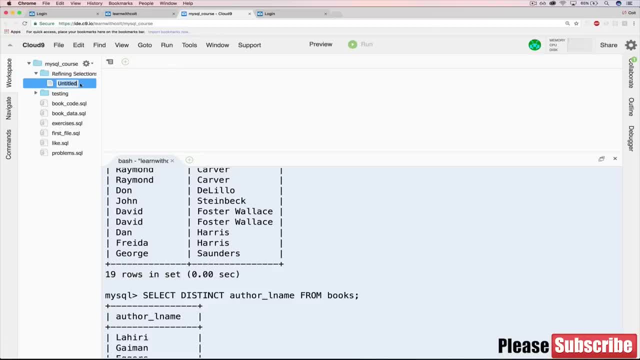 So I want to make a new file in that directory And I'll just call it distinct dot SQL, the most important part. Okay. So in here right now we have our select distinct author L name from books. So let's start off by just running this: make sure that our file is working. 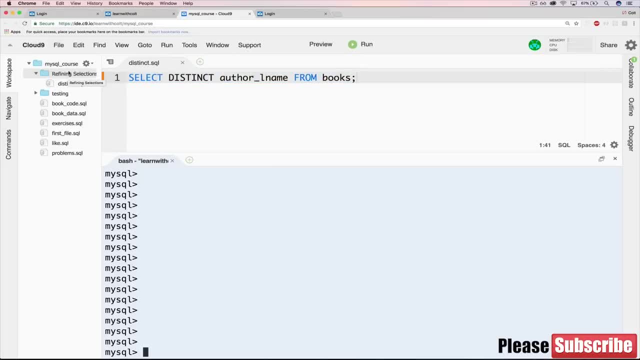 One thing I will point out. I don't recommend putting spaces in your directory names. It's just not a great idea. So I'm going to edit that It won't break anything. We can still do it, But it's just not great. 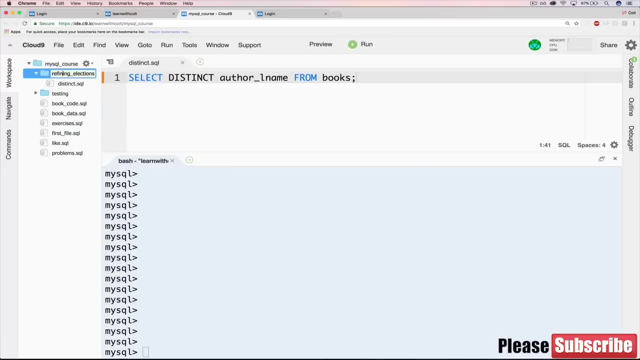 Let's just do like that: Refining elections- Well, that might work too, but refining selections- Alrighty. So if we want to run it, it's a source refining underscore selections: slash distinct dot SQL semicolon And it works. 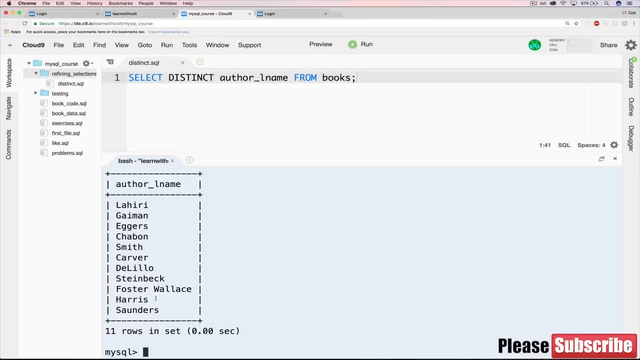 Okay, So back to the problem at hand. We actually get just distinct authors- first name and last name. So what we could do- I'll comment this out for now- is a select, and then we can concat author first name and author last name, just like that from books. 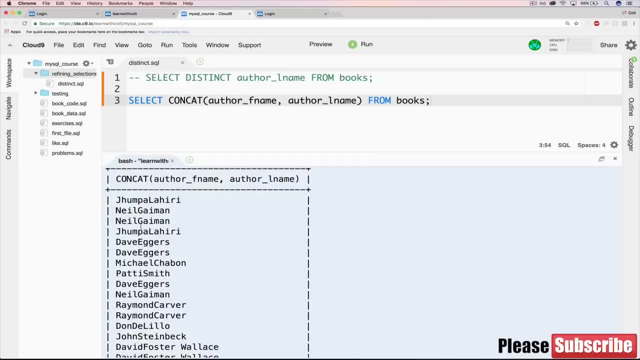 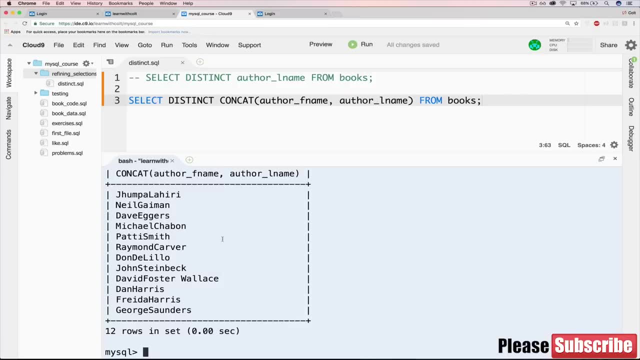 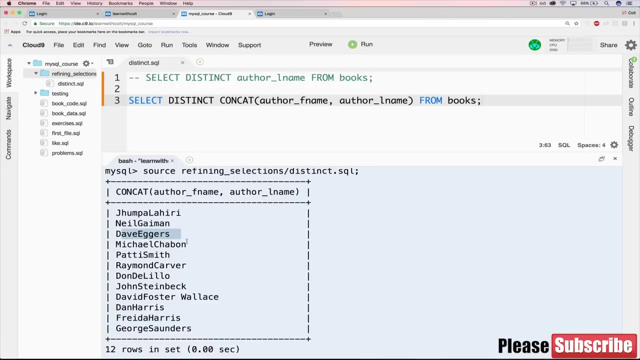 And if we save and run that now, we get this. And if we try and do distinct on that whole thing, Okay, That works, We get. Dan Harris and Frida Harris are distinct And we only have one Neil Gaiman, one Dave Eggers and so on. 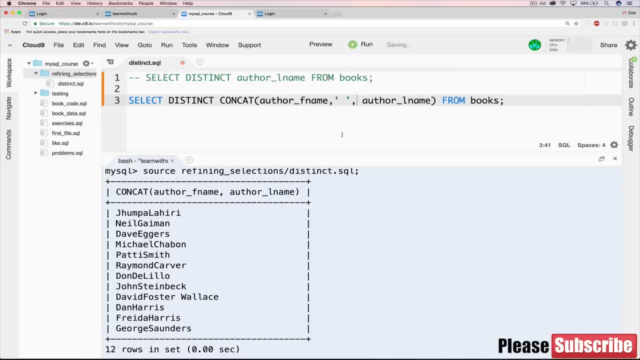 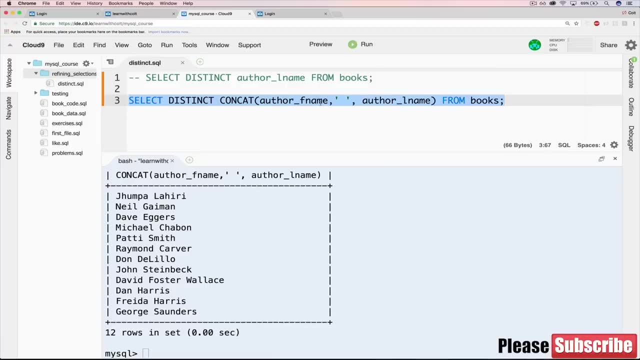 And of course we could go add the space that we want there and try doing it again, And that gives us distinct full names like this. That's one way, but there's actually an easier way And that's using distinct. We just do a select distinct. 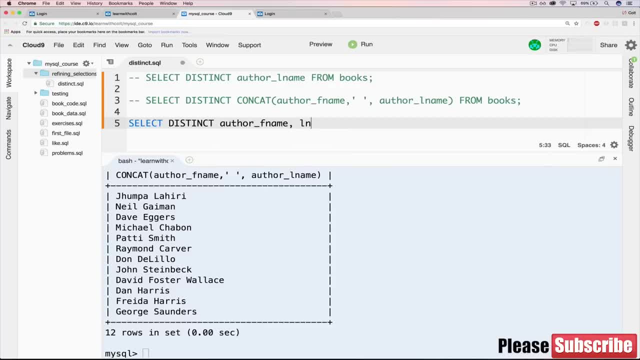 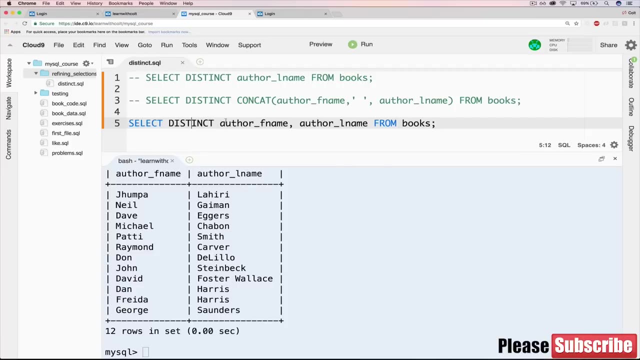 And if you do, author, Okay, First name first or L name, just separate them by a comma And we try running that. now You see, we only get unique rows back, So it's basically applying distinct to the entire row. So in this case it's basically saying I want the combination of the first name and. 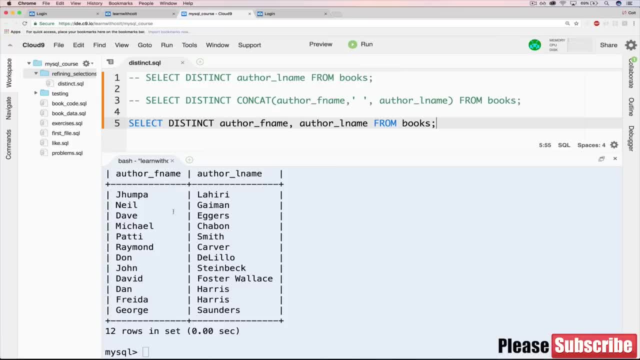 last name to be distinct. So that's why we end up with one Neil Gaiman, one Dave Eggers and one Dan Harris. Okay, And then we add another one Dan Harris and one Frida Harris. So it works in that way. 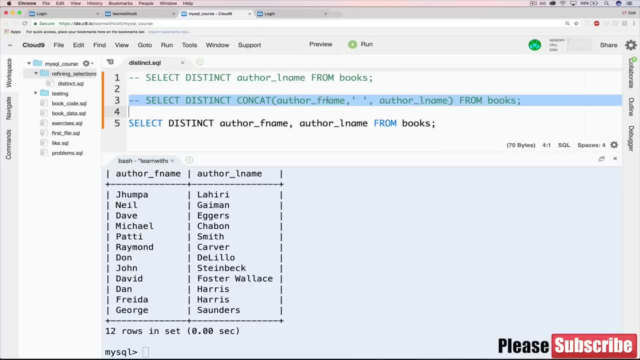 The only difference here, aside from this being longer, is that here we're actually just combining them and checking if it's distinct. here SQL is doing it or my SQL is doing that for us, And it depends just how you want your results printed out. 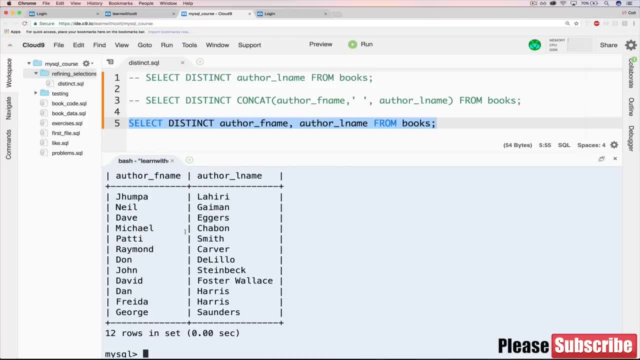 If you want them combined as a full name, then this method works better, And if you just want to keep your data separate in two different columns, then this is much easier and a little bit shorter. All right, So that's pretty much all there is to distinct at its core. 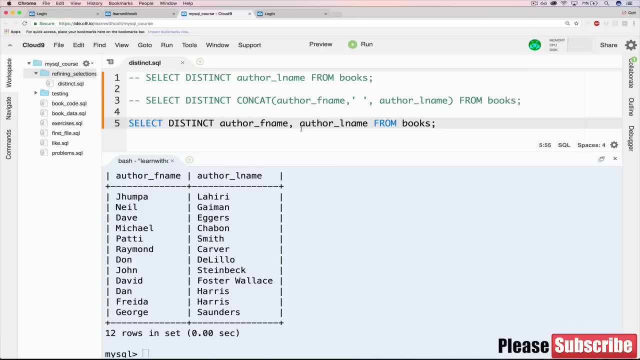 It's pretty simple and it's powerful too. It's something we'll use quite a bit throughout the course. As our data gets more complicated, we'll also have more duplicated data, which isn't a bad thing, But sometimes, when you're trying to understand it or work with it, you only want 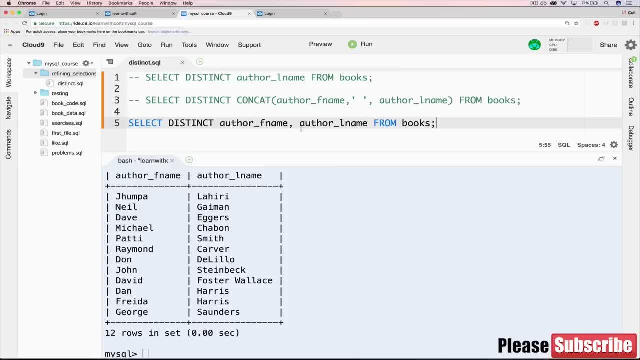 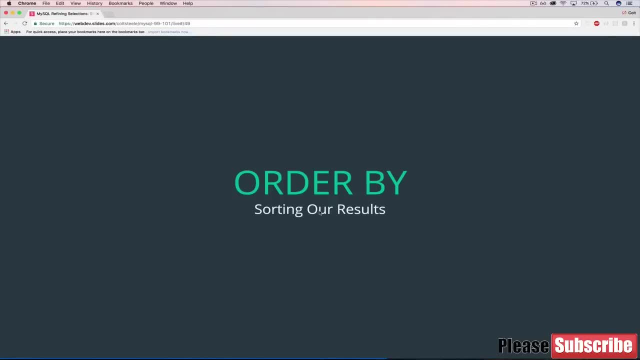 distinct data, So you use distinct. All right, I should shut up Moving on along to our next topic. I guess that's okay, Moving on along. I'll keep using that. Our next topic here is order by. So, as a subtitle tells you, it's how we can sort our results, which is something that we'll want. 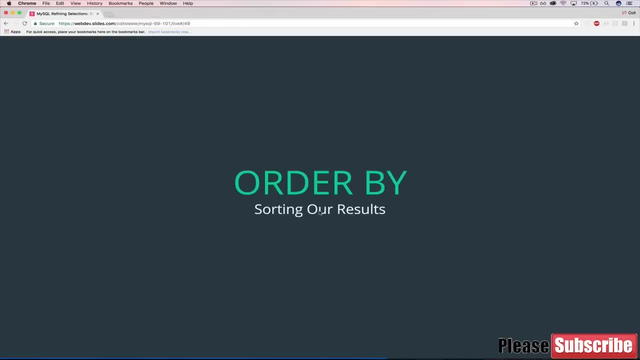 to do. Hopefully you see why that's useful. when you're trying to understand things. It's good to be able to sort your data. So with our books, for instance, right now we're getting them all in the order that they were inserted in, And maybe we want to do things like find the best selling books. 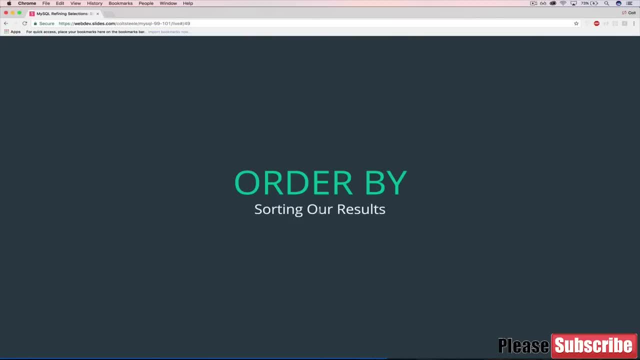 or the worst selling books, or find the most active users on our website, or the least active users, or something similar. Find the most upvoted posts or the post that has the most comments on our blog, or whatever we're working with. It's important to be able to sort things. And again, 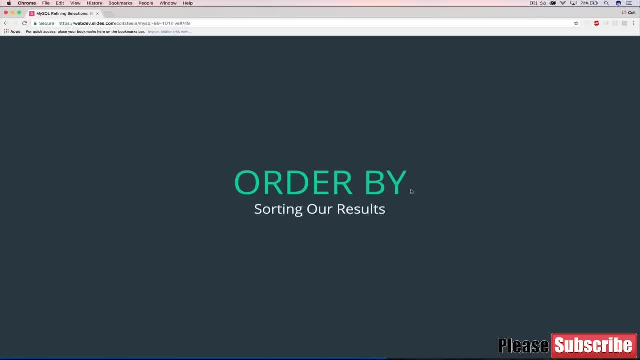 the way we do that is by using order by. So let's take a look at an example. Here's a query that's going to select all the author last names from books. So up until this point, nothing is new: Select author last name from book or books. But after that we add on this little thing: order. 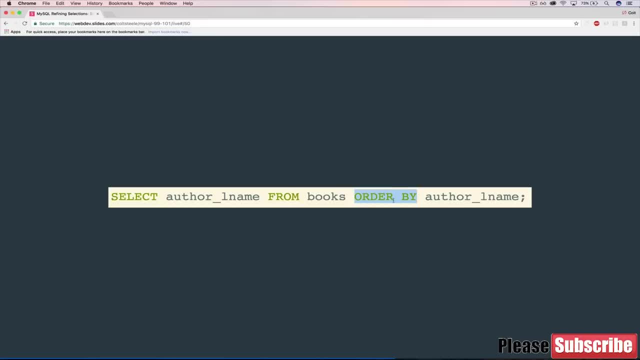 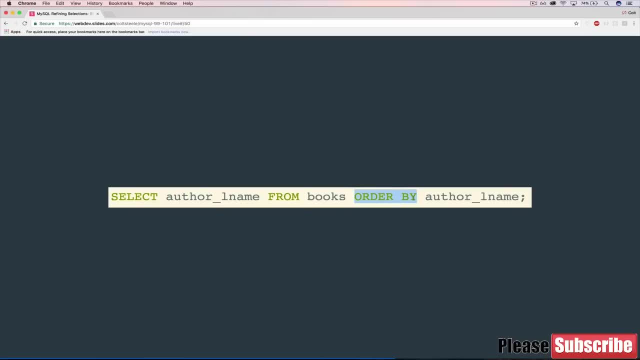 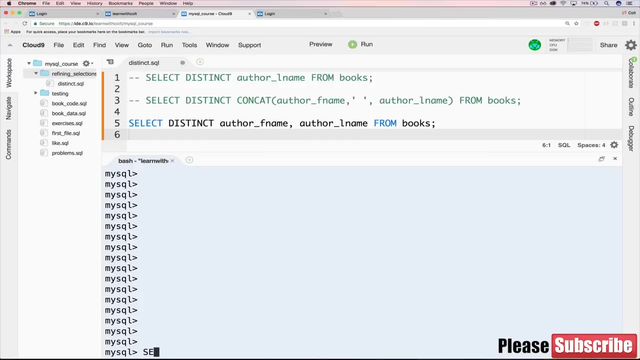 there's one word, or there should be an underscore, but there's a space or space by. And then what do we want? to order it by By the last name. So let me show you: If we go here, we just do a select. 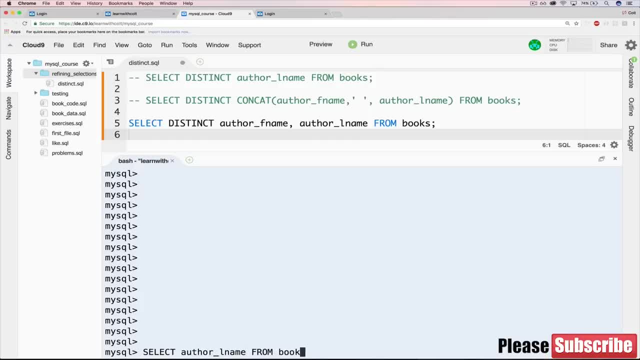 author L name from books. This should be review what we get. We get them in the order they were inserted, So that's not alphabetical at all. So if we want to do alphabetical, select author L name, order by, And then we have to say author L name, just like that. And as you can see, now we have 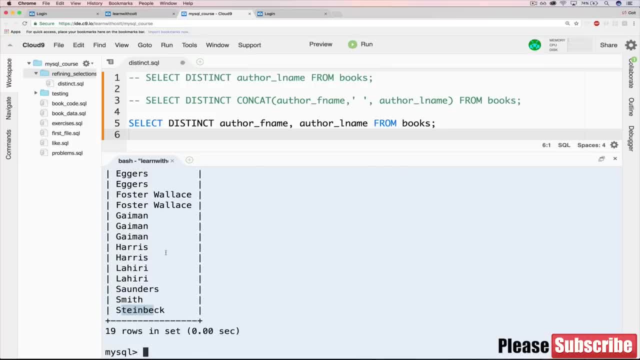 Carver up top all the way down to Steinbeck. And you should notice it is sorted by default in ascending order, So from C or A technically down to Z, And it's actually alphanumeric as well. So if we do titles, for instance, let's just do select title. 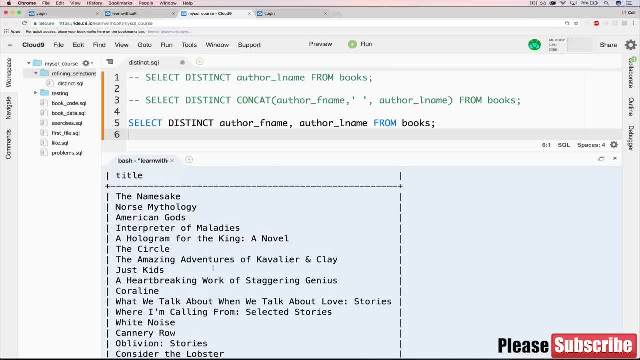 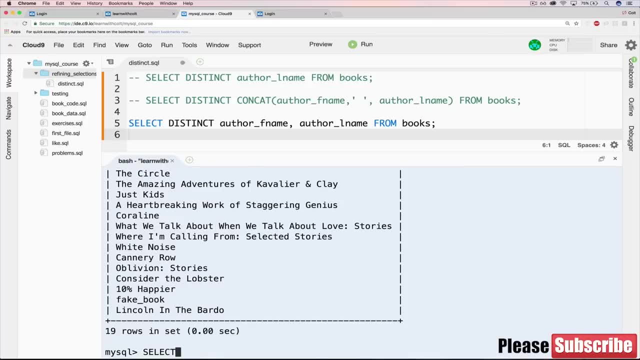 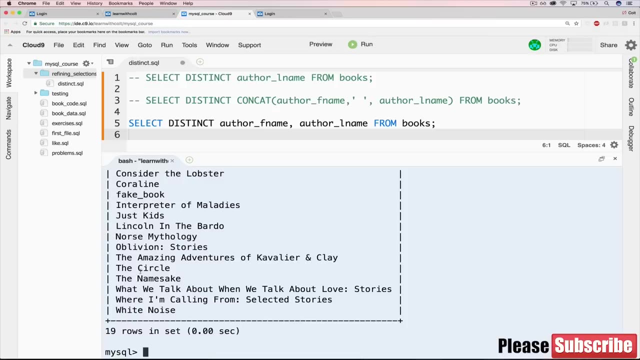 From books. We've got a title that has an A at the beginning, but we also have 10% happier. So if we do this- select title from books, order by title- you'll see we get the 10% happier first. 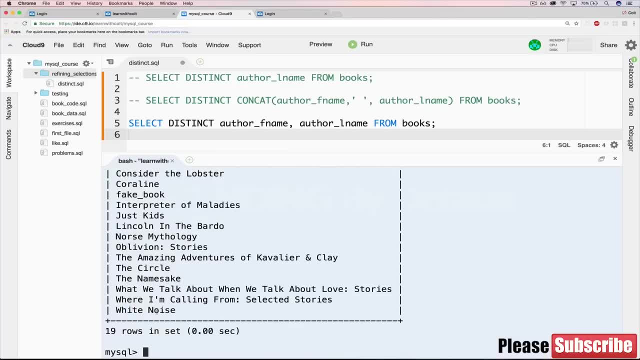 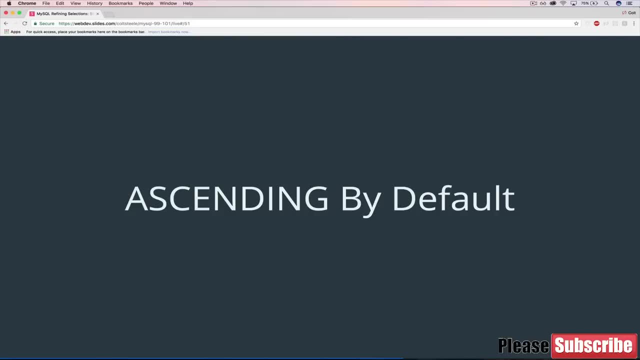 before the A's and all the way down to W. So, as I mentioned, it is ascending by default. So if you don't specify an order, it just assumes you want ascending. But of course we can change that, as my slide says, by just providing one thing at the end. So everything up until this point is the same. Select author L name from books. order by author L name space: DESC. And in my opinion this is also something that's kind of confusing because it's DESC. But then the abbreviation for ascending is ASC, which is only three letters versus four. But that's just my opinion, So let's try it now. 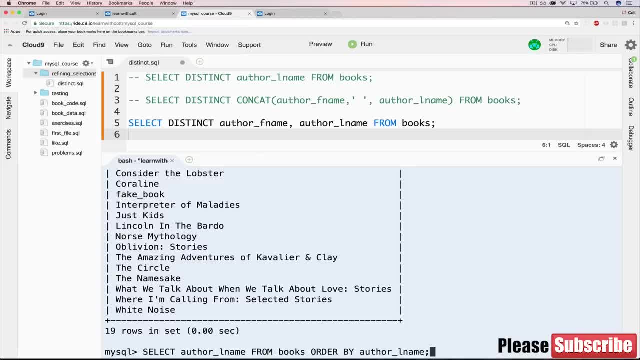 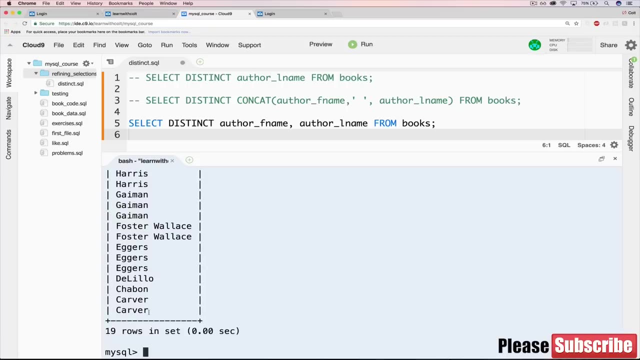 Now, if we recall what we had: select author L name from books. order by author L name. There we go. This is the original in default ascending order. But if we add DESC, you can see it's reversed. Now it goes from Steinbeck down to Carver. Or if we do the same thing with our title and we just add on DESC, it now goes from white noise down to 10% happier And of course order by will also be the same. 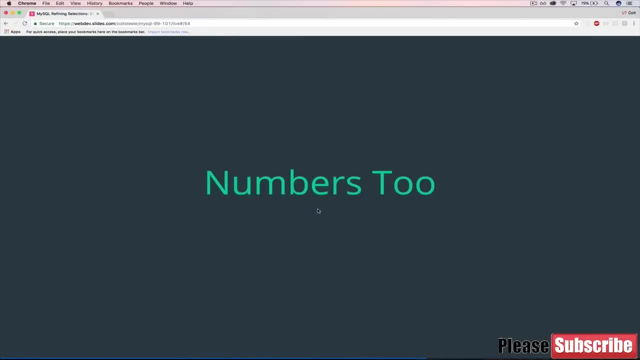 We'll also work with numbers. So it's pretty common that we want to sort things numerically, whether it's the number of orders, or the sort, the highest priced items or, like I said earlier, sort the blog posts by whichever have the most comments, most to least, or something like that. Those are numeric values. So to do that, it's the exact same syntax. All that we change is what we're ordering by. So, in this case, released year, which is 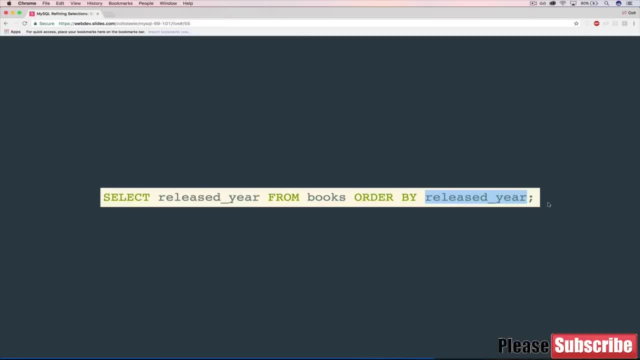 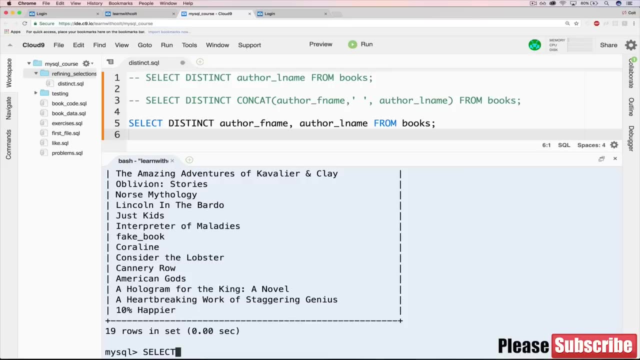 So, in this case, released. So in this case, released year, which is an integer, select released year from books, order by released year. So let's try it out, Let's do a select released year from books without the order by. And they're in all sorts of crazy order. I think our lowest one is 1945, all the way up to 2017, which is that Lincoln and the Bardo book Definitely recommend it. still So if we recall that line and just add on order by: 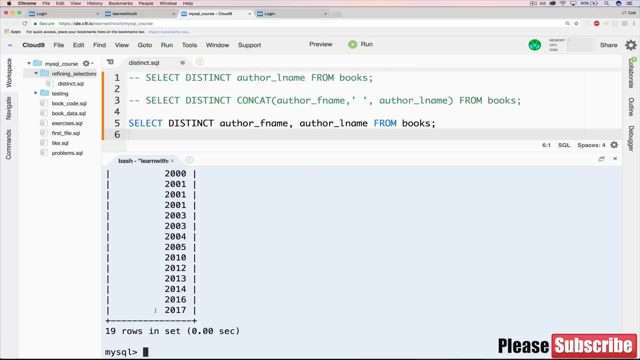 released year. There we go And by default it's also ascending: 1945 up to 2017.. We could reverse it with DESC, just like that. And just to prove to you you can do this, You can be explicit with ASC ascending and get the same order if you left it off. 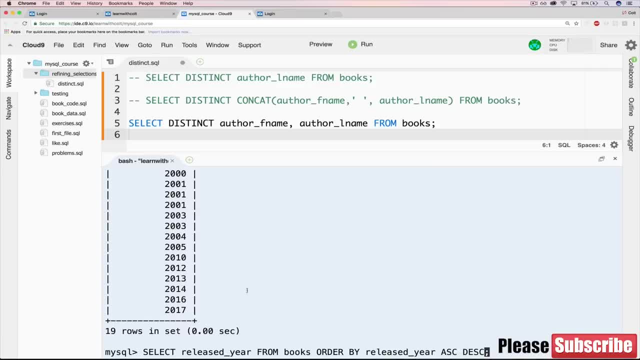 And not to harp on this too much, but I just I don't like that letters. it's just, it should be consistent. so if we leave it off, though, we get the same results. okay. so that's the basics of order. by another thing I'd. 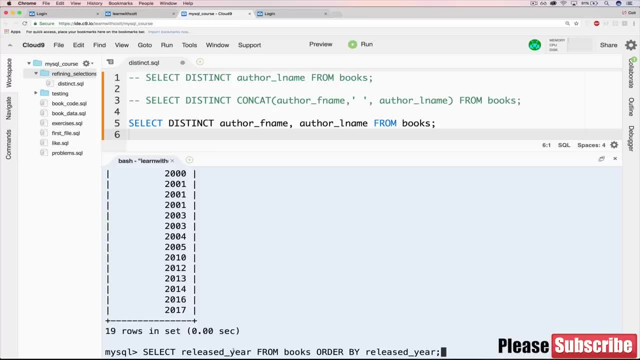 like to highlight here is that we've been doing things like select released year, order by release year, where it's matched. what we're selecting is matching how we're ordering it. you don't have to do that. so let's say we wanted to get, let's say we want title and year released here, that is, and pages or not. 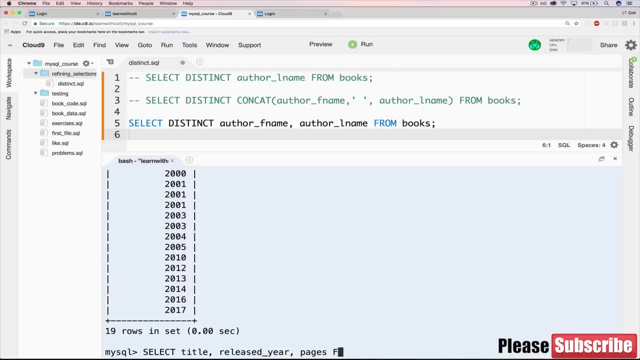 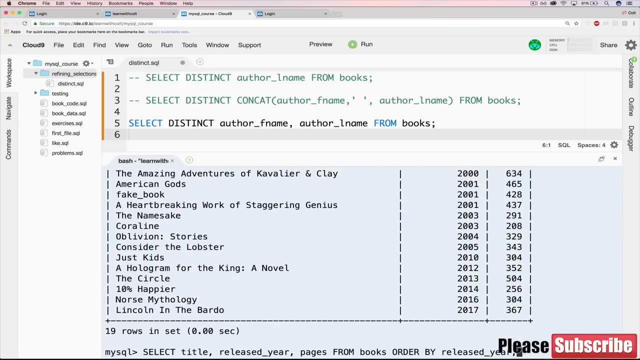 and I want all three of those from books order by and we'll do released here so I can do that and it's going to order them by the release here but still gives me all the data. so it's not like you know. it has to match. 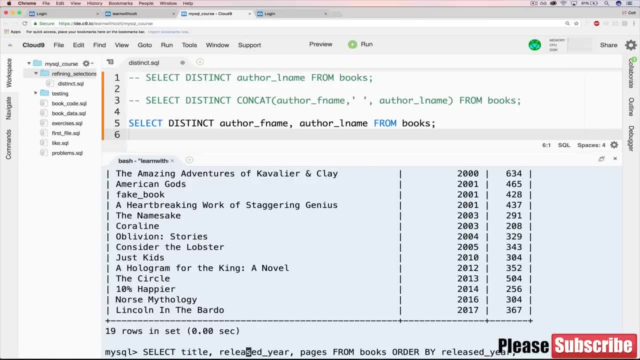 you know it has to match. so it's not like you know it has to match, or I could even leave released year out of this entirely. I don't have to select it, but I can still order by. so I could select title and pages and order by the. 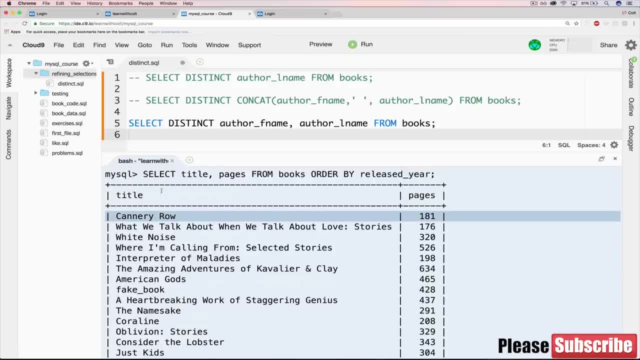 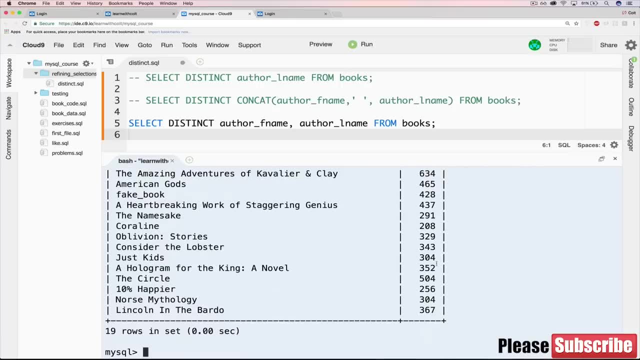 released year. you can see: the first one we get is canary row and the first one we got here is canary row from 1945, and the last one was Lincoln in the Bardo 2017. last one is Lincoln in the Bardo 2017. 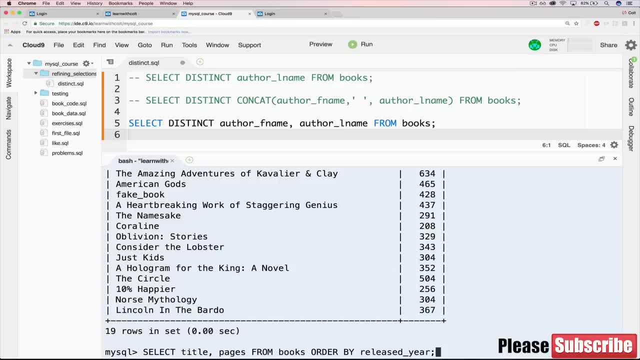 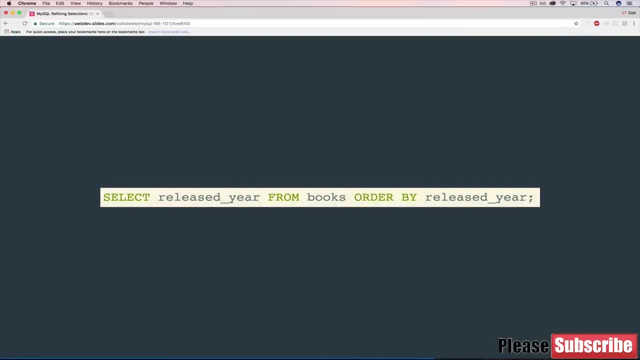 even though we don't have the year actually printing out. so that's all I want to show there: that you don't have to be ordering by something that you're selecting, or that it doesn't have to be the only thing that you're selecting. so here's another little quirk: of order by, if you take a look at this query- select. 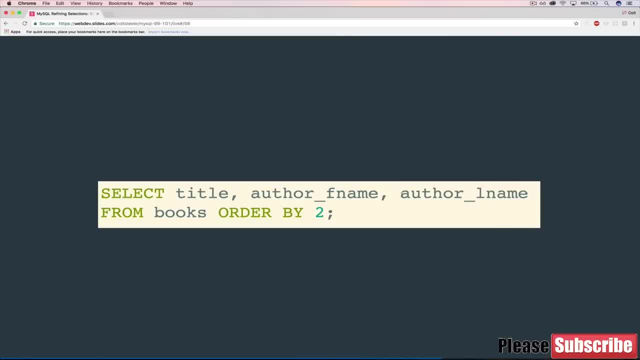 title: author F name, author L name. and I put this on two lines here, not because it's correct to do that, but just so that it's easier to read for you. so select title, author F name and author L name from books. order by two. what do you think? 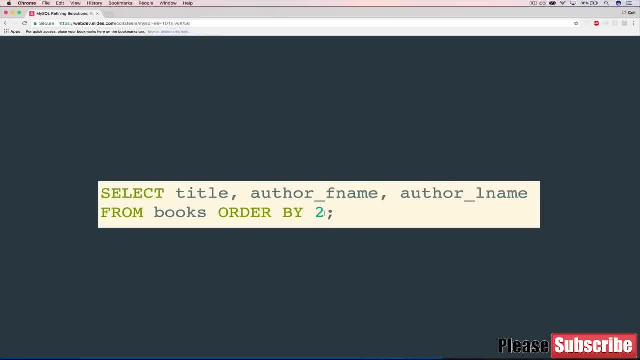 the two refers to. well, in this case it's actually just a shortcut, so we don't have to rewrite author F name and author L name and then we can just go ahead and select title, author F name and author L name. so if we're selecting title, author, 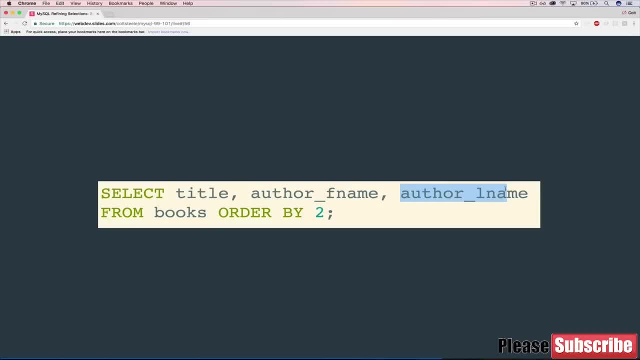 F name and author L name. this will be one, this is two and this is three, and it's a shortcut for me to say order by two: author F name, so let's copy it over. try running it. you can see the results we get back. they're not sorted. 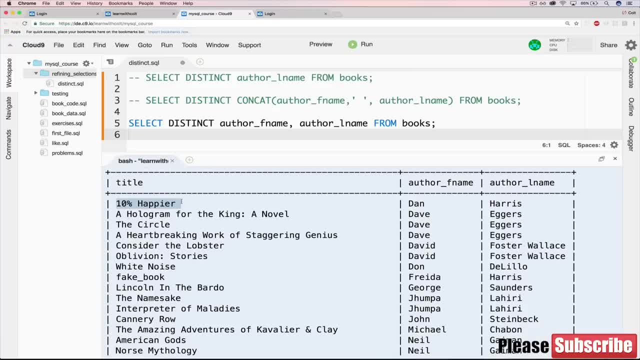 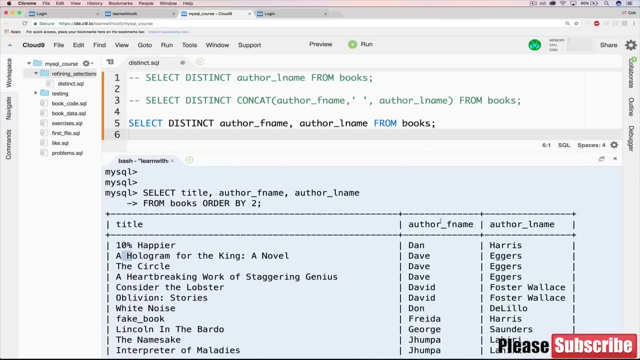 alphabetically here, even though sort of looks like it, because we have 10% happier and then a hologram for the king, 10 and then a, but it's not the rest of the way, it's not. but you can see over here we've got Dan first and then David. 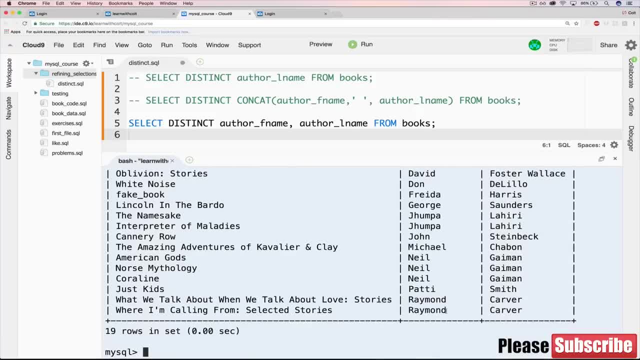 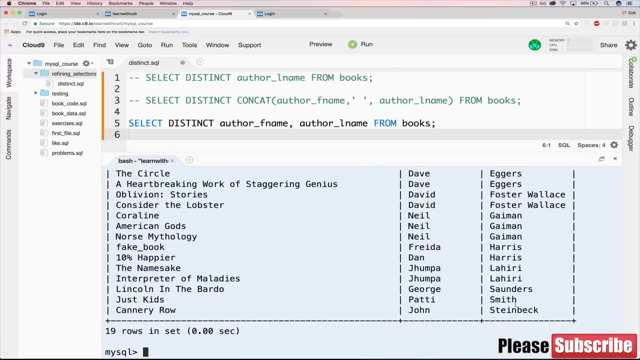 Dave, data, Don freedom, blah, blah, blah down to Raymond. and if we wanted to sort instead by last name, we just change it to three again, because author L name is the third thing that we're selecting. and now we go from Carver down to Steinbeck and likewise you can change it to one to sort by title, and we could also switch. 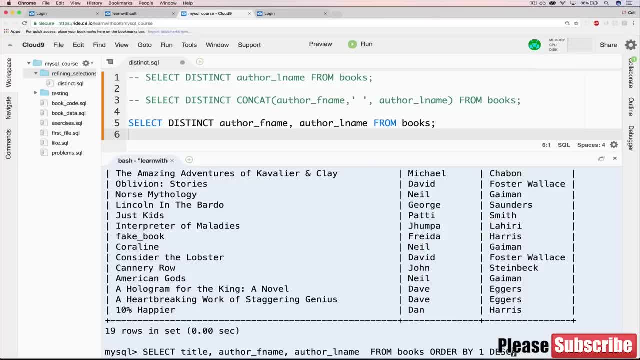 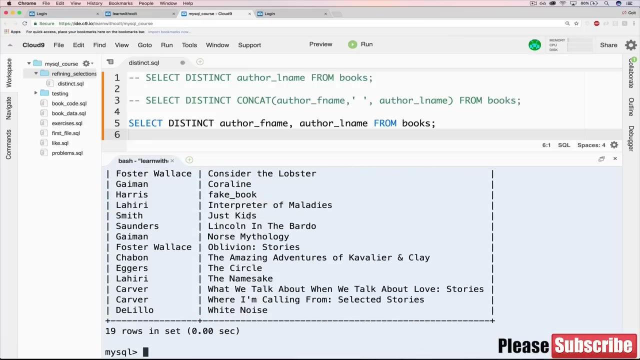 it over to descending and that works, and if we did switch the order here, just to show the order does matter. so if I do, author, L name, comma, title. if I want to sort by title, I would need to do two now, and now they're sorted by title. okay, so 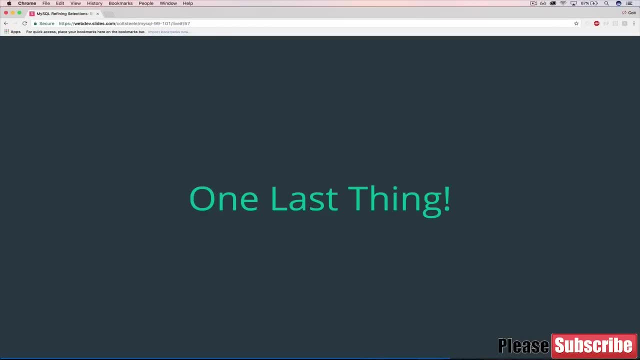 there's one last thing, and I made a slide to remind myself about it, which is here. so what we can actually do is sort by, or order by, two different columns, which seems like something that you wouldn't really do that often- and, truth be told, it's not, but I just want you to know that you can. so, to show you what, 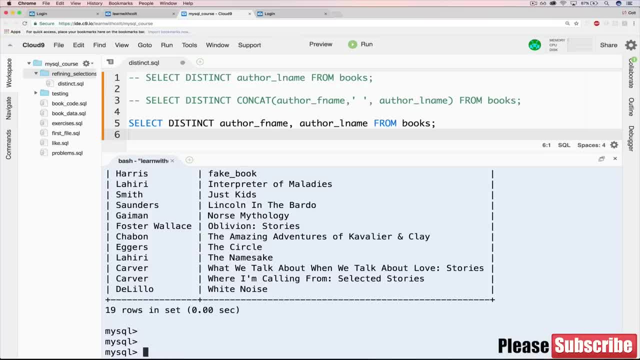 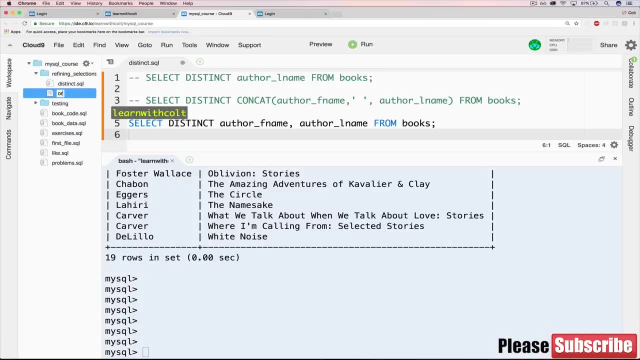 I'm talking about. let me first do a select and I'll make a new file for this one as well. just because we're gonna have a little bit of code, let's do new file. I'll just call it order underscore by dot SQL. okay, and if we do a select: author F name, comma author L name from books, just like. 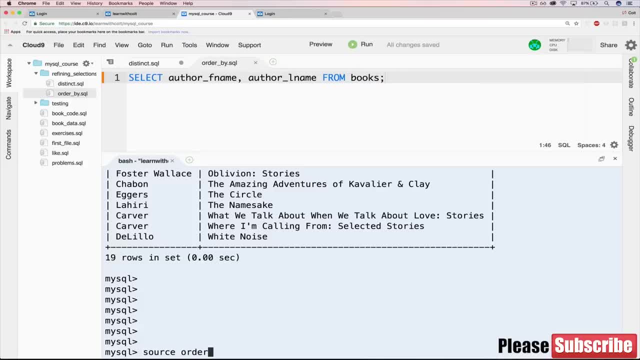 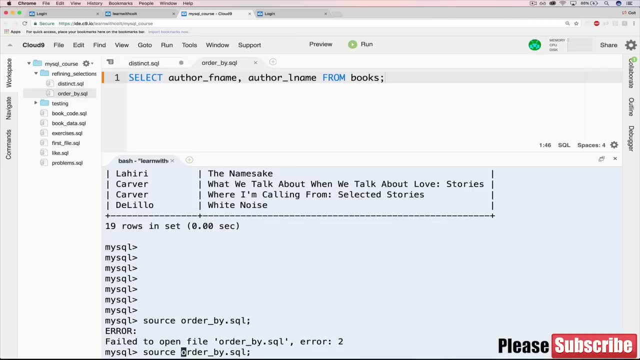 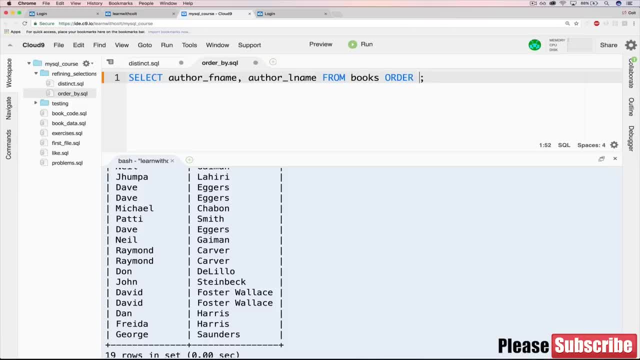 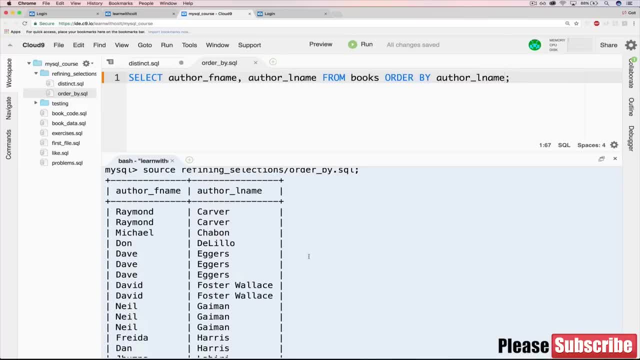 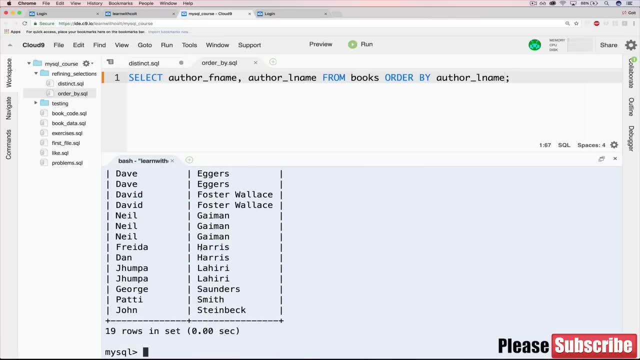 not sorted. so now if I do an order by author last name and I read it, everything looks good. we have our author sorted alphabetically- carver game in Harris. but then that's where we run into our problem, which is Harris and have the same first or the same last name, and we want the entire author name to be sorted. 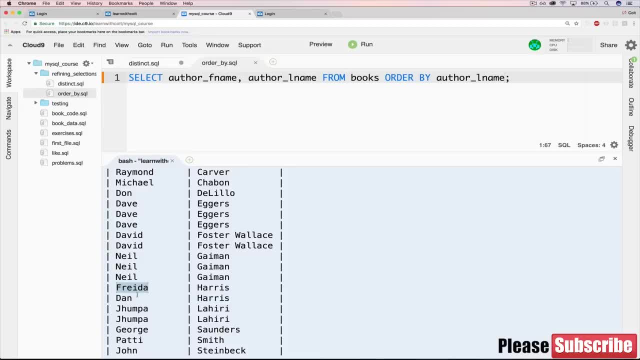 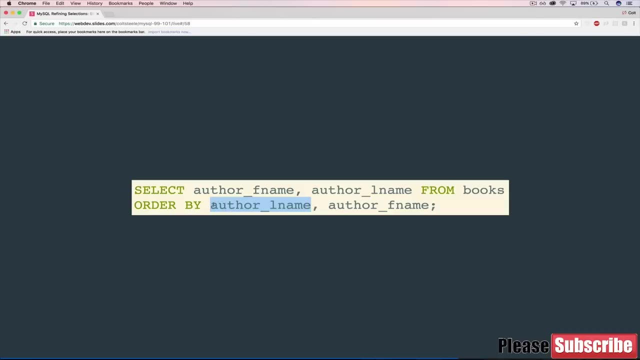 alphabetically. well then, we need to go to the first name, and in this case, frida harris is in front of dan harris, even though d comes before f, so we want dan to come before frida, and that's where this comes in handy. we can sort after. we sort by last name, then sort by first name. so it's. 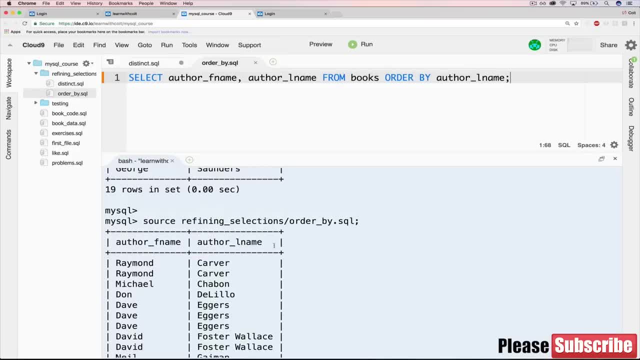 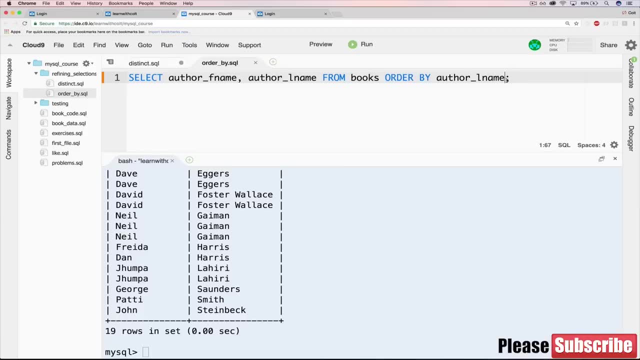 not going to redo everything. it's going to keep basically the initial sort and then sort first name. if there's any conflicts, so we can just add that in as a comma: author f name and save now, if you just focus here, so we have frida harris and then dan harris and if i source that and run, 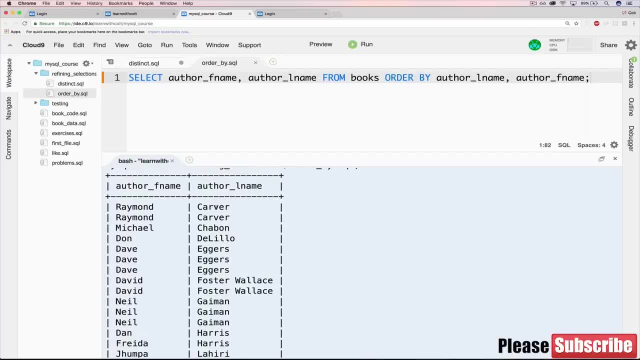 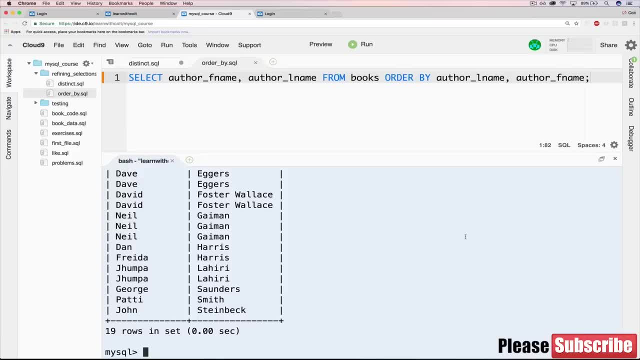 lot there. it's a little bit dense. i apologize, but order by is useful. like i said, you'll be sorting lots of things and it helps you understand your data, especially when we're talking about sales data or site. you know site specific data. there's a lot of insights that you can get just by putting. 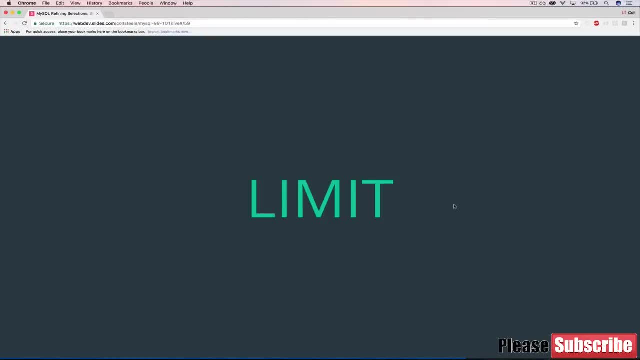 it in an order. next up in our toolbox is limit. so limit allows us to specify a number for how many results we want to get, and then limit allows us to specify a number for how many results we want to get, and then limit allows us to specify a number for how many results we want. 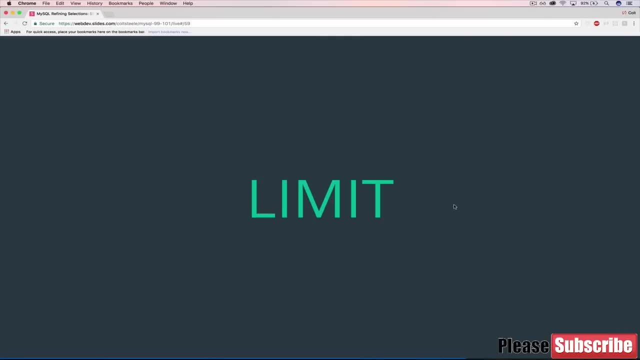 to select. so i could say things like: i want the first two best-selling books rather than all best-selling books or the top ten most recent books. so we often use it in conjunction with order by or sorting, because that typically is going to give you something meaningful rather than just saying: select all books and give me the first two. well, how is first defined and we can do that. i'll show you that. if we do a select, let's go ahead and click the select button and we're done. and now we're going to know we got two of them that are our best selling books, so we are going to know which ones are in order to buy. if we select both, then 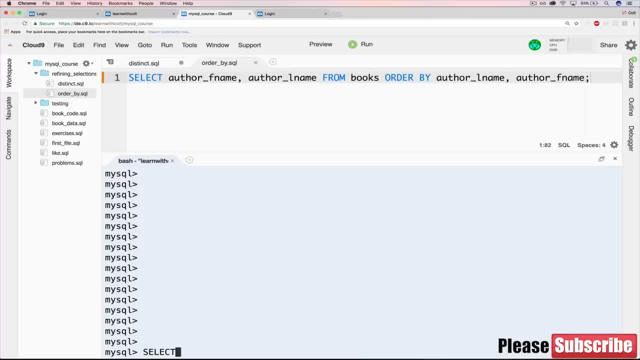 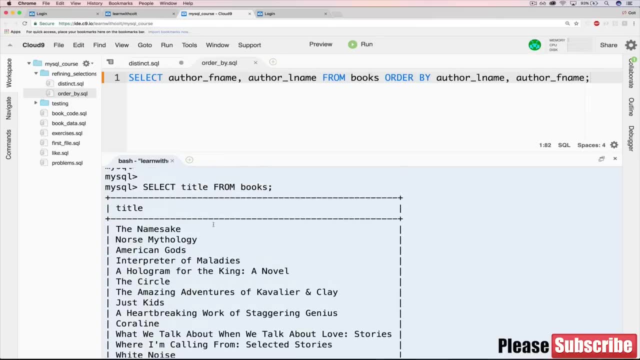 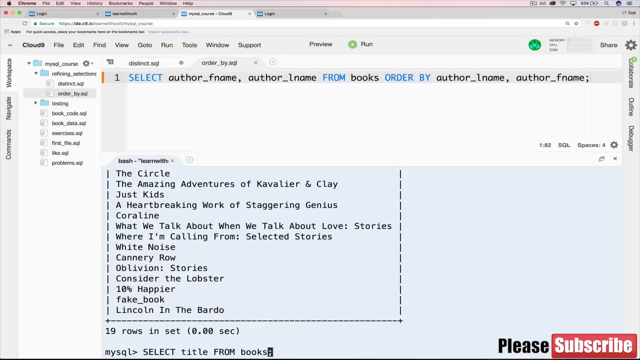 first defined and we can do that. i'll show you that if we do a select- let's just do title from books, the order that we get them right now again, is the order they were added, so we have the namesake norse, mythology, american gods and so on. so i could limit this and the 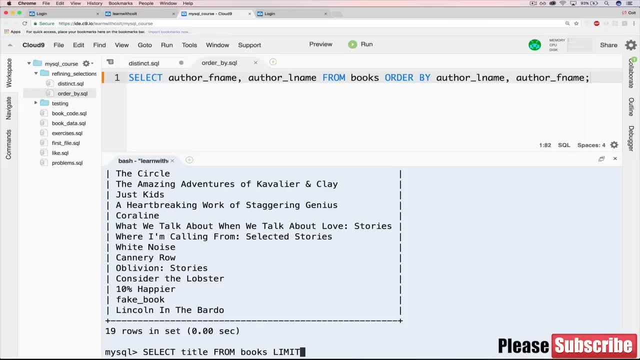 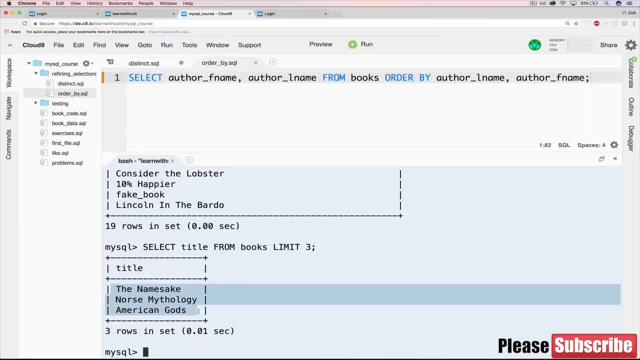 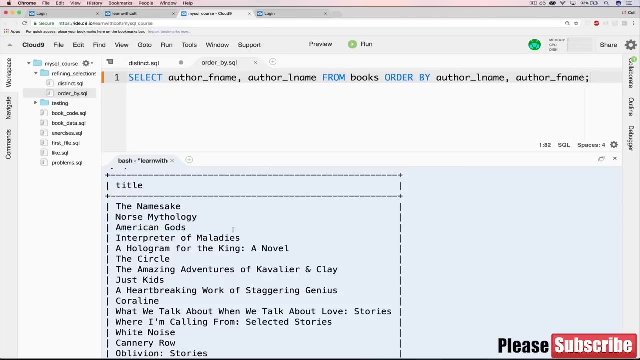 syntax looks like this: i just add limit at the end, just like we added order by limit. let's say three, and now i just get those first three. so it's going to limit it to the first three. whether they're sorted or not, it doesn't care, it just chops it off right there. so again, it's not that. 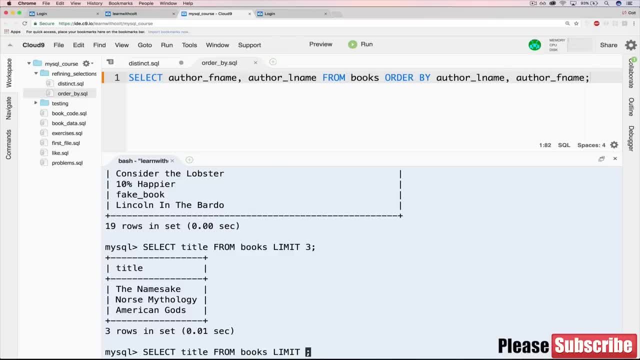 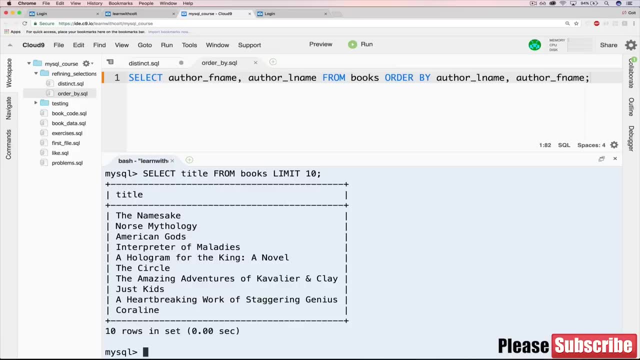 useful or that meaningful, just to do it on its own, like this. but we could do, you know, limit one, limit 10 and so on. uh, and that's basically all that there is to limit. you know, we can do it with a select star. if i only want, let's say i want- everything about the first book, there we go, i get the namesake and 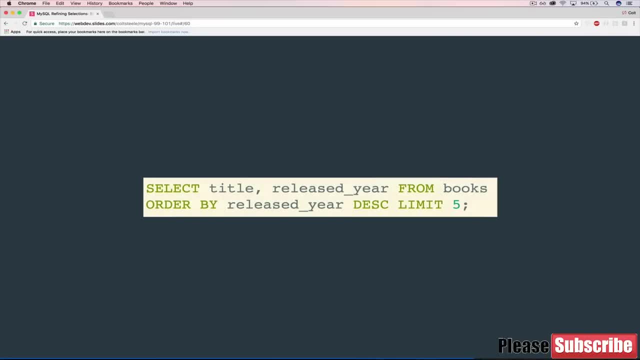 there's everything about it, but more often than not we're using it with order by. so here's an example: if i want the five most recently released books, i'm going to, and i only want the title and the release year in this case. so select title and release year from books, then i'm going to. 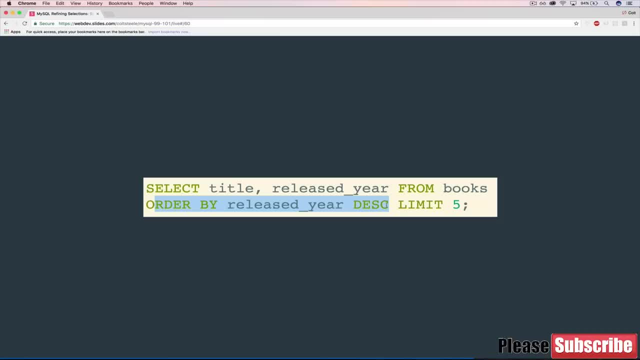 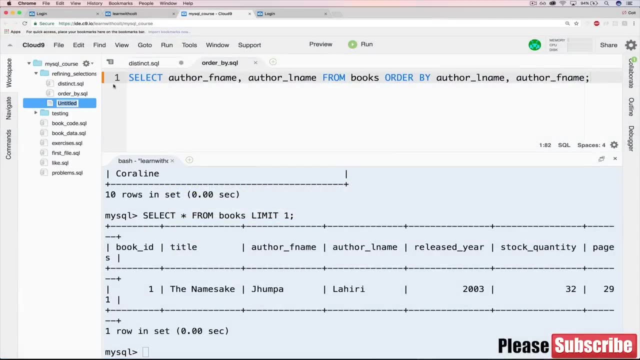 order them by the release year descending, and then i'm going to limit it to the first five. so let's try it. i'll go ahead and make a new file again, limitsql, and in there i'll write a select title, comma, released year from books. i won't add limit yet, let's just make sure our source is working. so we'll do a source. 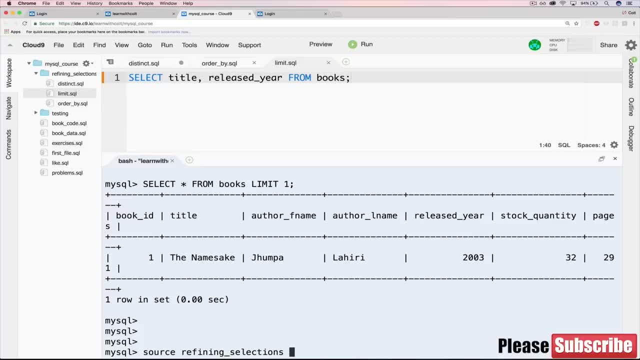 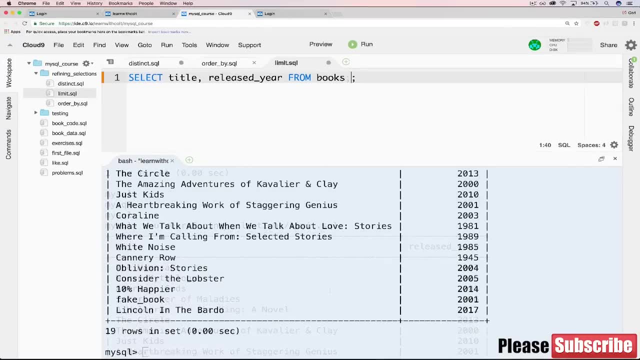 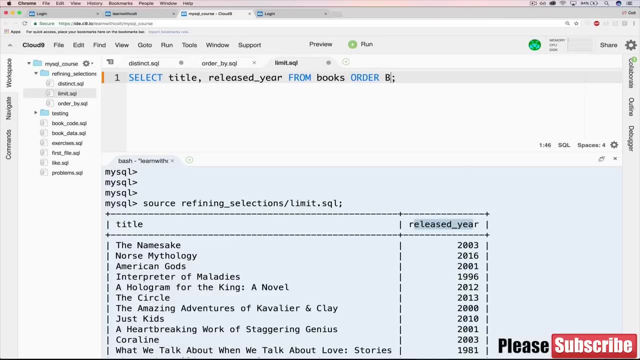 refining- why did i name this so long? refining selections, slash limitsql. fortunately, you only have to type it once. okay, so that's working. so now what we'll do is order them by that released year. so we'll do an order by and we could write release here, and i will, because it's more specific or it's it's easier. 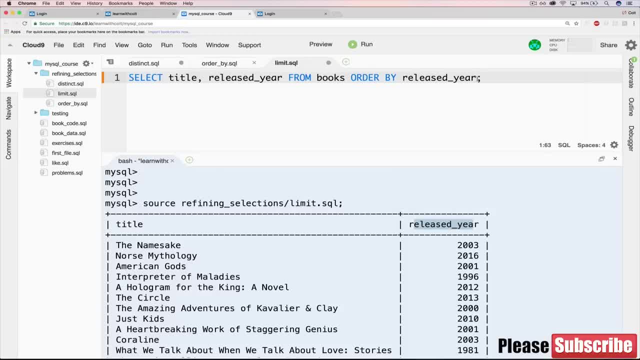 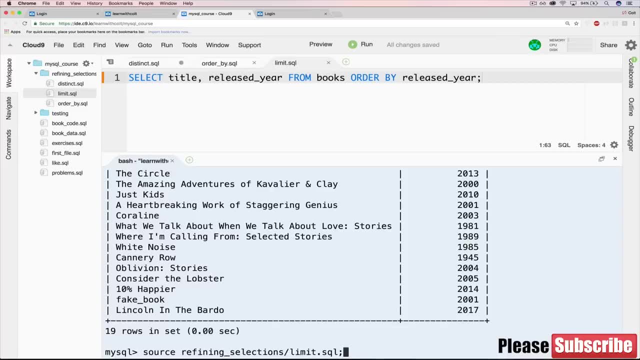 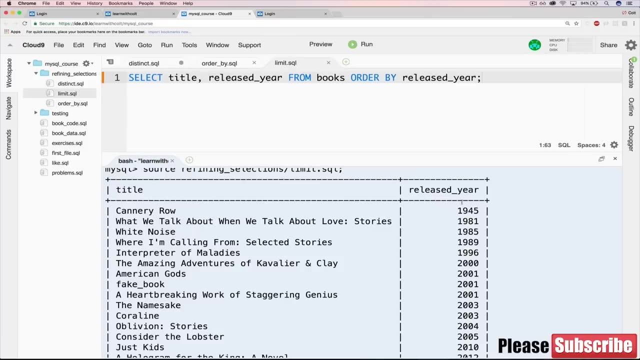 to understand. it's more semantic to write it out, even though it's longer, but of course we could replace it with two, as we just saw in the last video. so order by that release year. if i do that now, that gives us all the books ordered in ascending order based off of their year, which is not what we want. 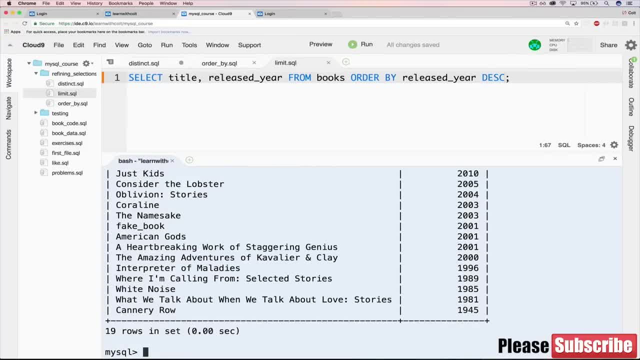 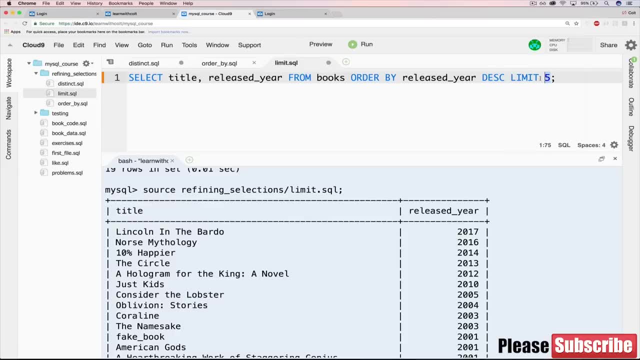 so we can switch that with desc. there we go, and now i can limit it to five, and so that limit comes last as well. so it's going to do everything and then chop it wherever you specify. so that's important to know. so let's try it now. make sure i save, and there we go, the five. 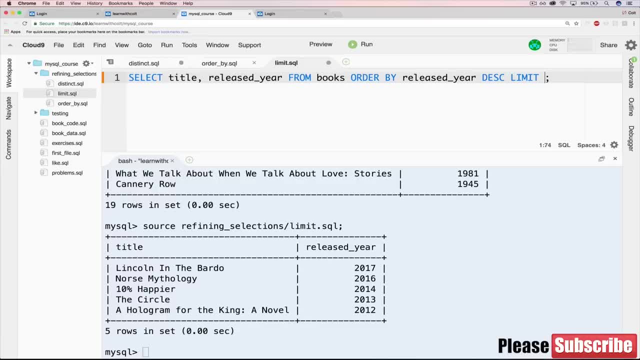 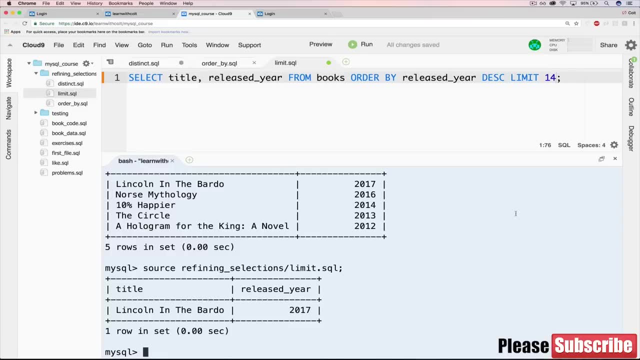 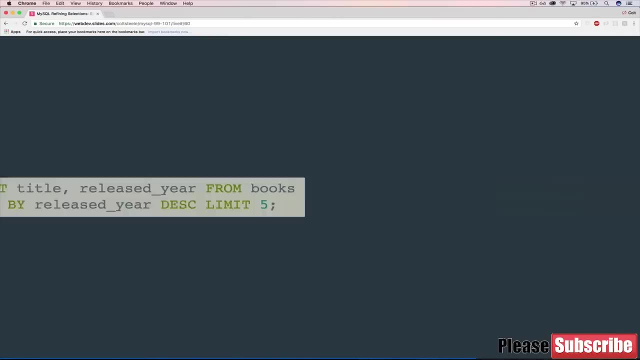 most recent books, and, of course, we can change this to whatever number you want. if you want the one most recent book, or if we wanted, let's say, 14, we can do that. so there are a few other ways we can use it. for example, here's the same query. however, i've written it slightly different, so everything up. 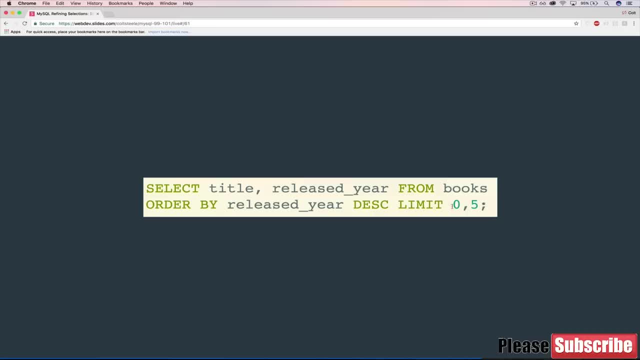 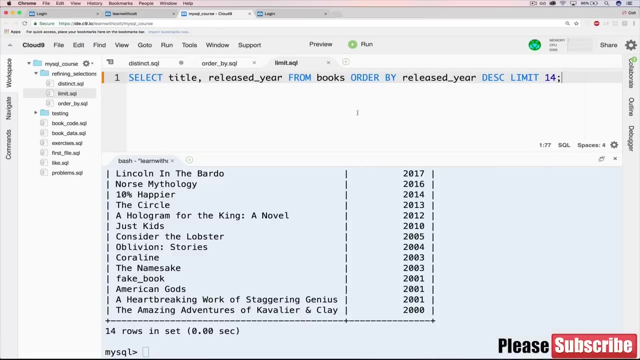 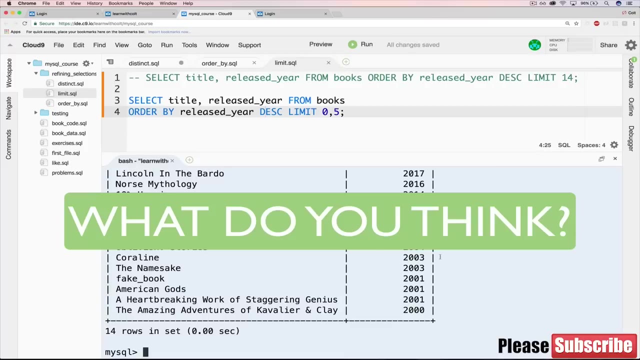 until this point. right here is the same limit, but this time i'm saying limit zero, comma five. so if we just copy this, i won't make you watch me type that whole thing out, and i comment this out and i try running this. now just take a guess: what do you think will happen? 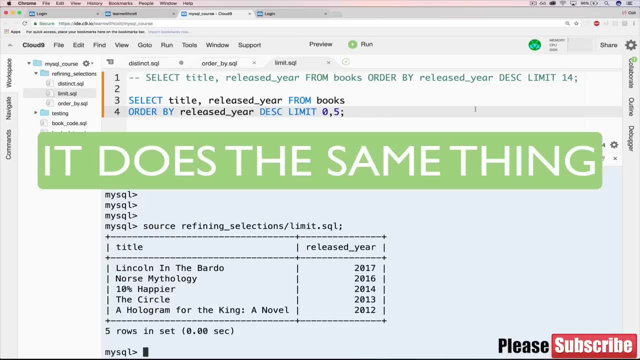 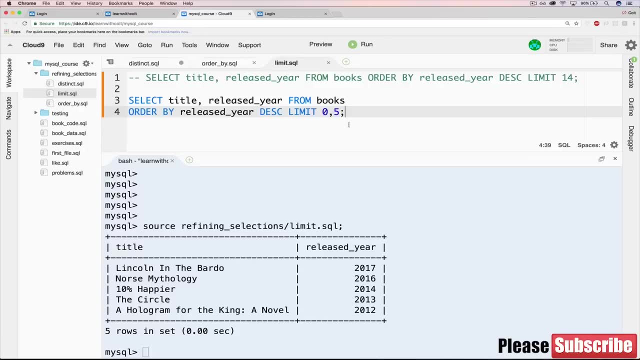 and here we go. it does the exact same thing. so this is a syntax that allows us to specify a starting point and then how many we want to go from there. so basically it's saying- and this is kind of confusing because, uh, it starts at zero, so the first row and a. 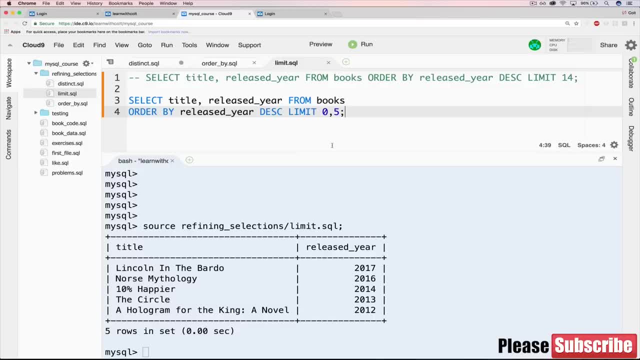 in a table is the 0th row, but then when we're dealing with strings, like when we had hello world, H is actually the first character, in mysql at least. so anyways, it's saying: I want the first row and I want to go for five rows, so we could. 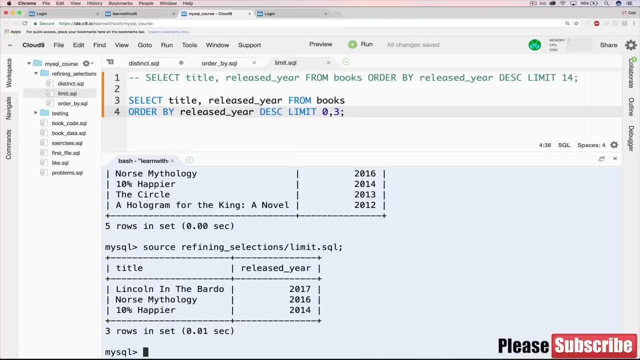 change that. I only want three rows this time. if we rerun it, it gives us the first three rows, but then I could shift it. let's say I want to go, I don't know why, but the second row onwards. so it gives us North mythology 10% happier and 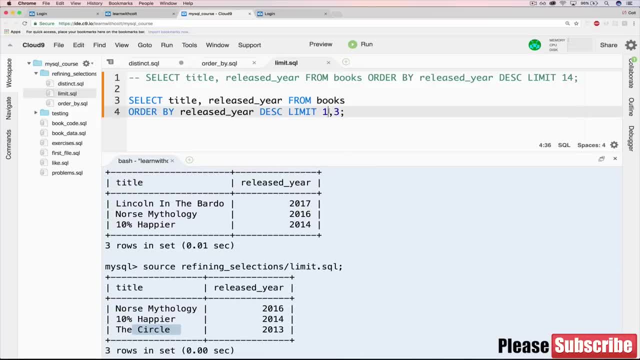 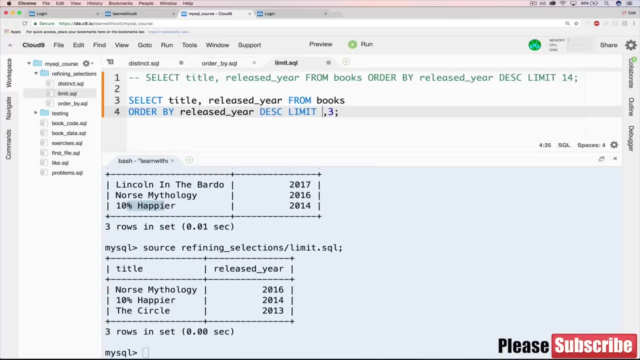 the circle. if you didn't catch that before, when it was zero, we got Lincoln and the Bardo Norse mythology and 10% happier. when I change this to one, it shifts the starting point. so it's not that. really it's not comment at all, but 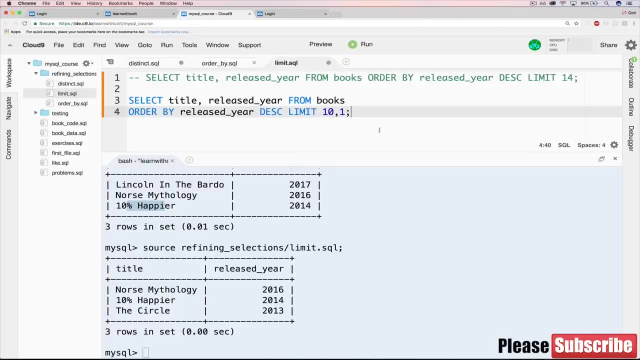 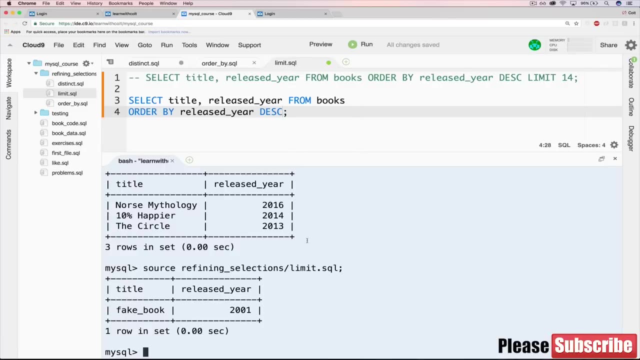 you could do things like 10, comma 1, and what this will do is go to the 11th book. well, I need to save first now. if I run it, it will give us the eleventh book. and just to make sure that we're right there, if we rerun it now, we could count down one, two, three, four, five. 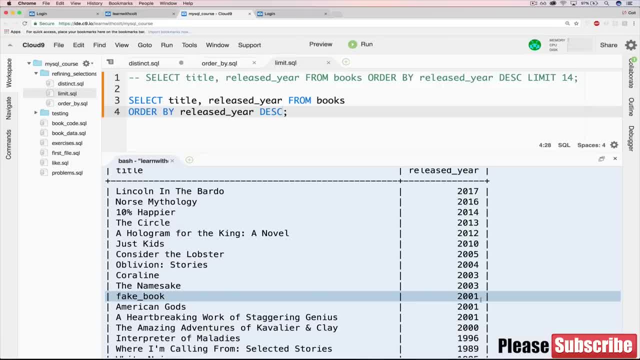 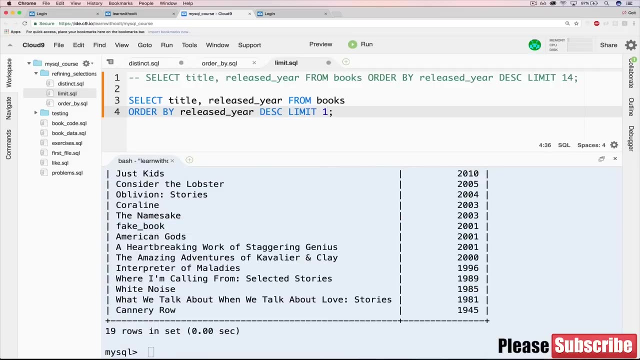 six, seven, eight, nine, ten, eleven and we get fake book. so if you need to access very particular rows based off of order, that is a way that you can do it. just honestly, not that common. pretty much every time that I use limit, it's in a context like this: limit one or the first three of the 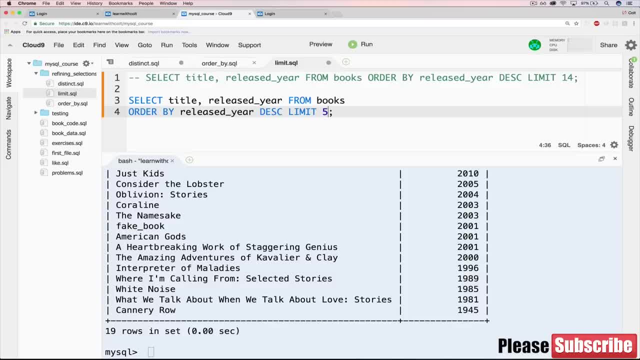 first five, something like that. but I'll give you an actual, a real reason you might use it. let's say that you have a blog site that you've created and your blog has thousands of articles in it already. when a user visits the blog page, you don't show them all thousand, let's say ten thousand results all at once for 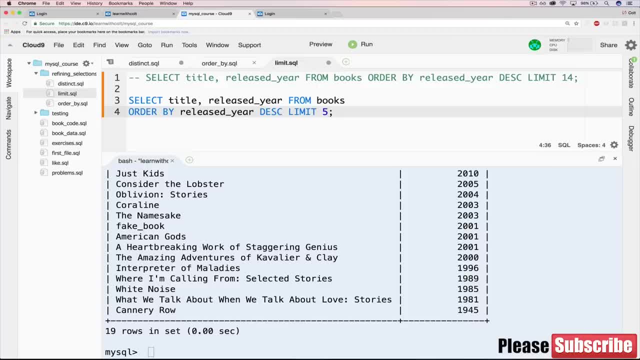 every blog post that you've written. that would be overwhelming and that's just there's too much information to display. most likely, what you'll do is have the first ten posts and then I can click a next button and it will load from post 11 to 20, and you know I can keep clicking next and so 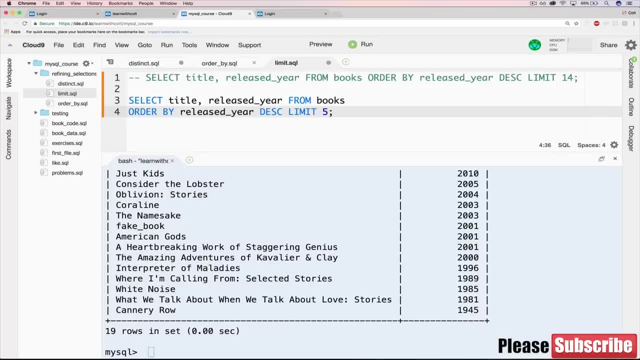 on. you've probably seen that before it's called pagination. so you can do that by, rather than selecting everything from your database, you could select from zero, and I only want the first ten, and then you're the next time through. you could select from ten and I want ten more, and so on. so that is a situation where you 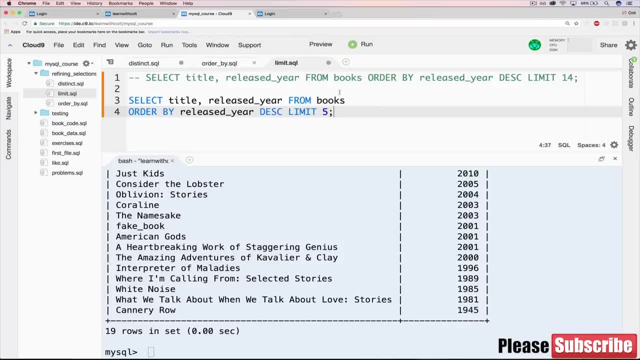 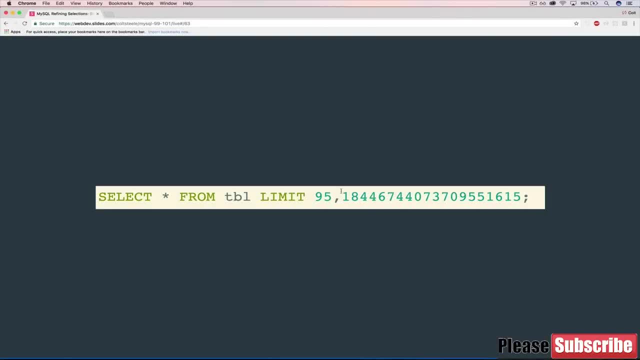 could use that limit and provide a range like that, but again, most of the time I just use this limit and then one number. the very last thing I'll show you is that this is actually straight from the Docs, from my SQL is. I think it's really clunky and weird that they even specify this. if you wanted to select. 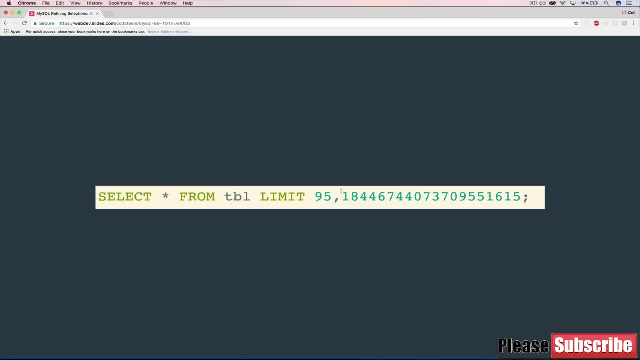 from one row all the way to the end of the table. so I want from row five all the way to the end. we might have however many thousand rows, there isn't a nice, elegant way of doing it. this is what you have to do: select star or whatever. 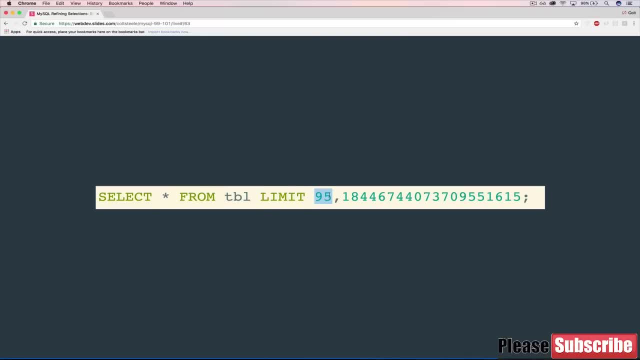 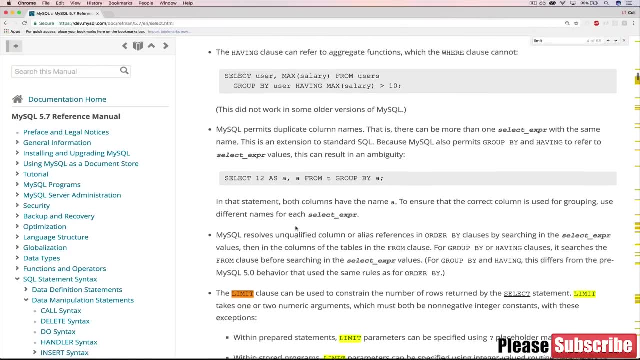 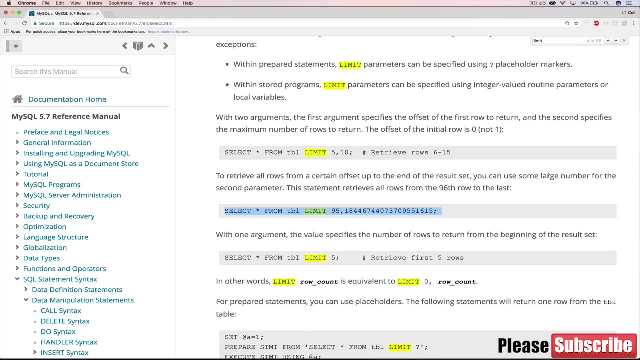 you're selecting from whatever table limit, and then you can use this as a way to limit and then, where you want to start comma, some gigantic number- and I'm not kidding, you actually have it in the Docs here, right? where is that right here? to retrieve all rows from a certain offset up to the end of the result set, you can. 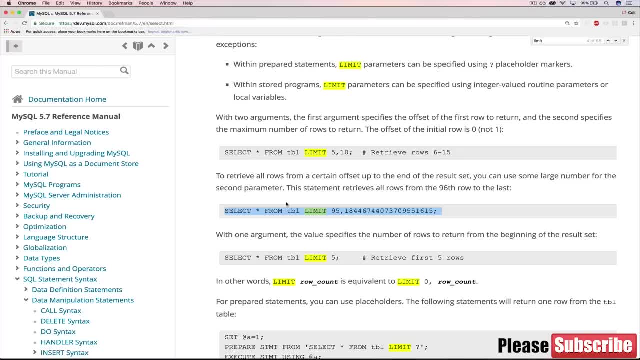 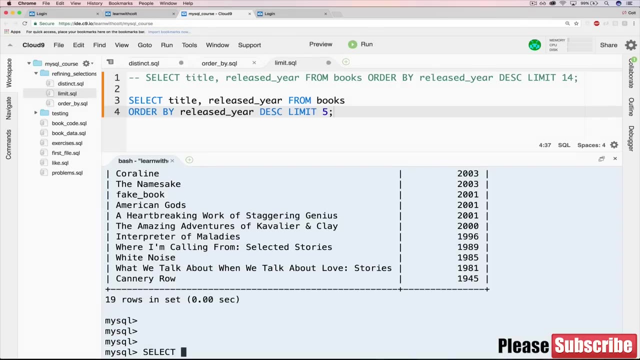 use some large number for the second parameter. so that's their official suggestion on how to do it. select star from table. limit 95 comma, some gigantic number that you would know. you never have that many rows in your table. so we can do that here if we just do a select title from books, order by, and let's just 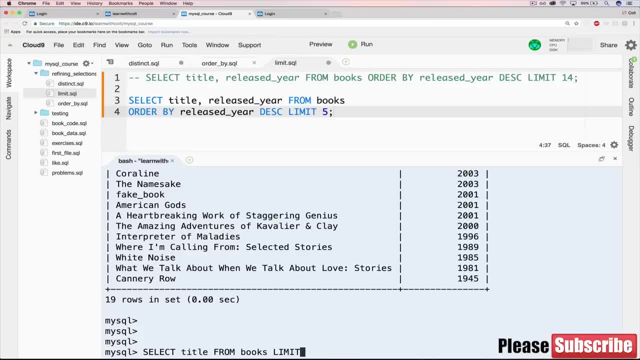 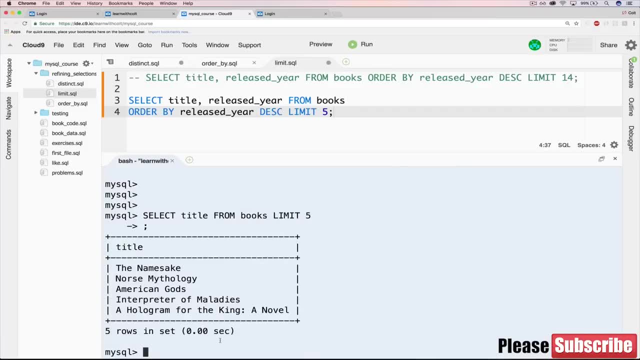 say: I want to go, we don't even need the order by. honestly, let's just do a limit. and if we just do limit five, that's gonna give us the first five. but if I want to go from five to the end, I can do limit five and then some gigantic number. 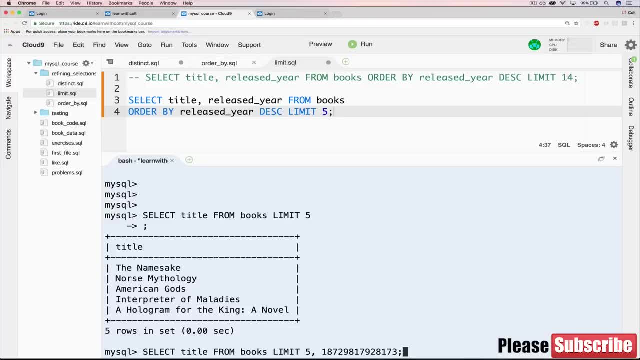 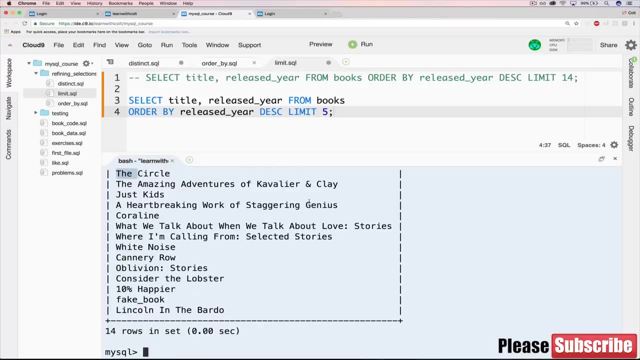 and in our case it doesn't even have to be that gigantic, so we don't have that many books. but if I do that, it gives us everything after five, or technically six, because it starts at zero. so I could reduce this down, I could just do like 50 and it. 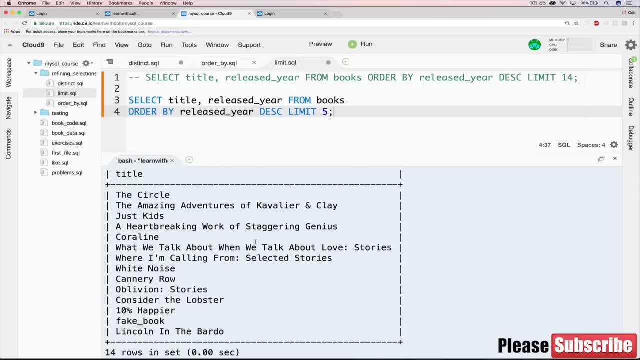 gives us the same thing because we don't have 50 books, so it just goes until the end. so that's it to limit, with all those weird things that I showcased and the odd situations and ways you can use it, the most common and the way that almost 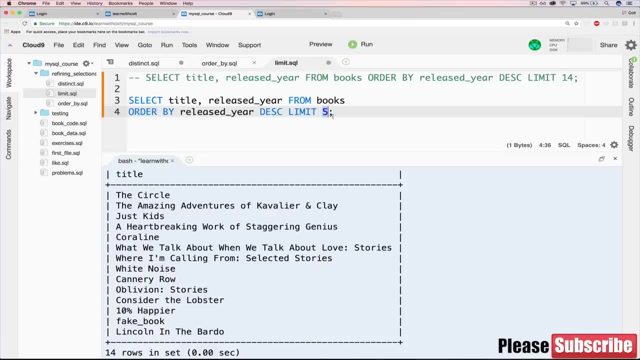 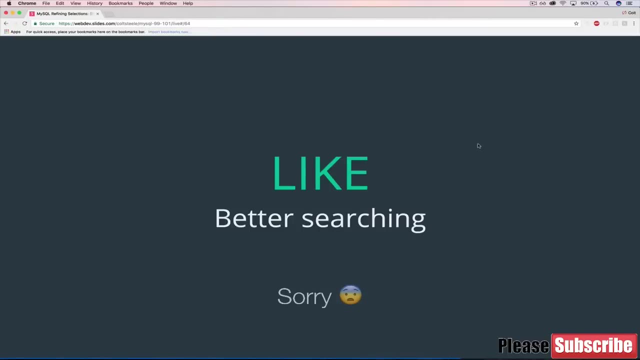 always that I use it. is this just limit? and then a single number, alrighty, so that's it, moving on to one more, and then we're done for this section at least we're not done with the whole course. all right, so we have one more video here, or at least one more tool for the toolbox, before we get to. 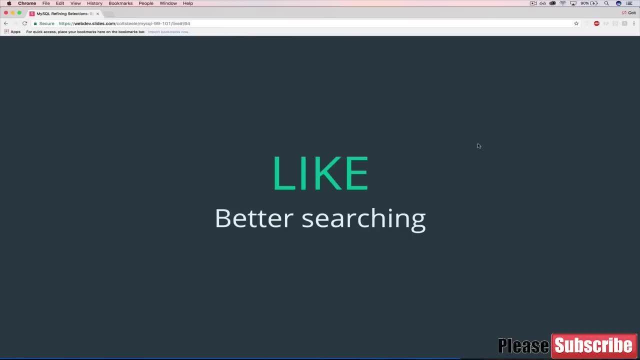 the exercise at the end of this section, and that tool is something called like, and I'll start off by saying like- is very useful. it basically allows us to perform better searching of our data. so if you think of when we saw how to use where, where would allow us to find exact matches, so I could do things like. 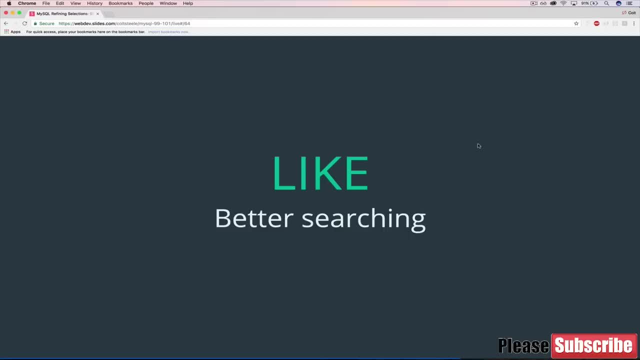 select star from books where title is exactly Harry Potter and the Sorcerer's Stone. but what if I wanted to select all Harry Potter books? I would want to do something like select star from books where title contains Harry Potter or starts with Harry Potter or something like that, and we don't have a way of. 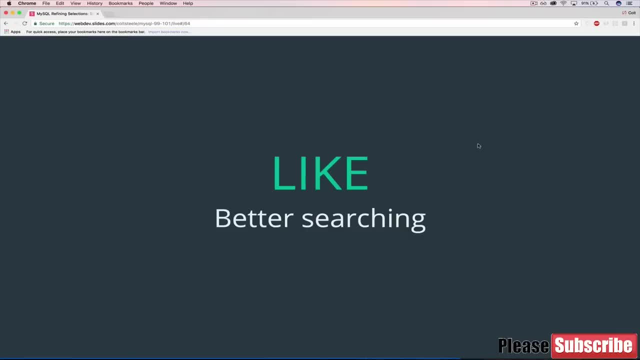 doing that. yet until now, with like so like, allows us to do things like this. imagine someone comes into your bookstore, if we have a bookshop, and they say: there's a book I'm looking for, but I can't remember the title. I think the author's first name is is David, or maybe it's Dan or or Dave. 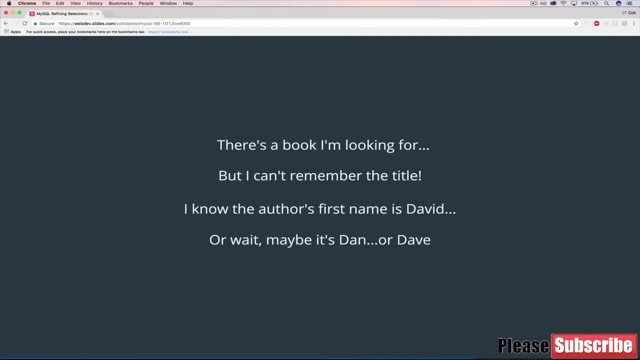 and you could go over to your system has a really helpful bookstore employee and you could just search for, let's say, books written by authors whose first name starts with da, which I guess is a very broad category, but you can still do that. if you search for authors at like a Barnes & Noble or popular bookshop or Amazon, you can do. 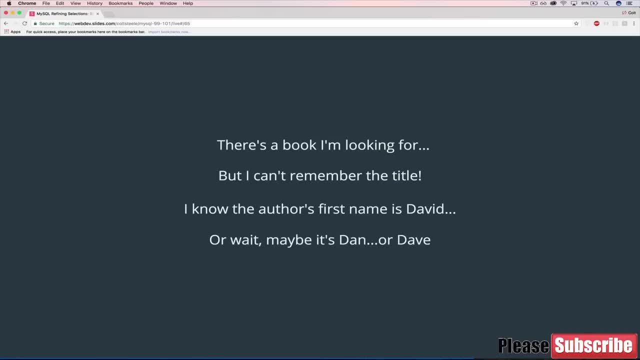 that type of search and it will work. it's just not that common. but we could do the same thing for books. like I said, Harry Potter is a good example where we want to search for all the Harry Potter books, not just the exact one word for word. match their character for character matched. so that's where where comes in. 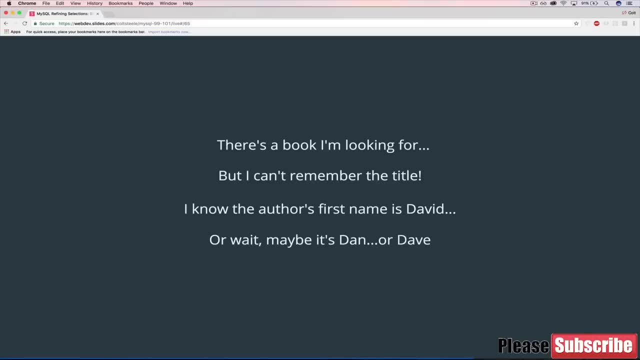 now you. it's gonna look a little bit odd when I show it to you, but that's okay. it's not that complicated. there's just some weird symbols here, so here's an example of using like: where so we? this is ignoring the first part of the query. 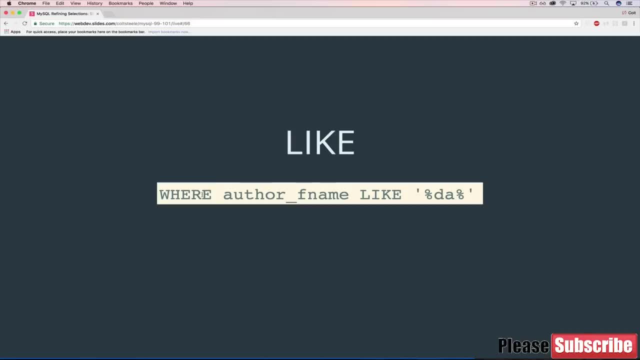 the select star from, or the update or the delete or whatever it is so blank where author F name like. and then in quotes I have this percent sign and da percent sign. so I'll tell you, first of all, what this is going to do is find where the author's first name has the letters da in it and these little things. 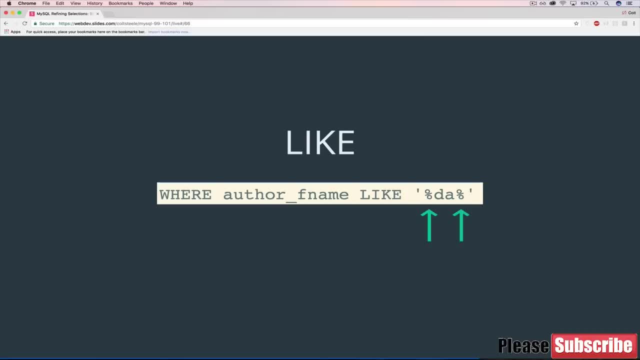 here those percentage symbols, kind of like that animation there. those are known as wild cards. so that's basically the way that we specify. we want to find author first names where there's something anything at all to wild card. so any characters and then these two exact character. 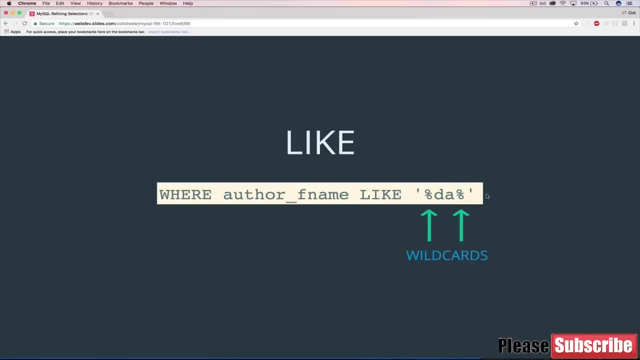 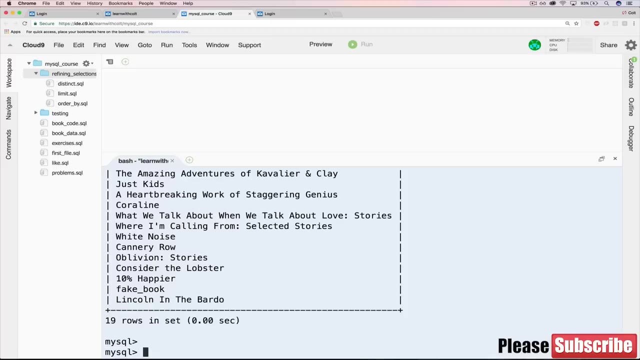 characters da and then anything afterwards. so it's basically a way of saying whatever blank anything da, and then whatever anything else afterwards. and if we try using this right now, actually you'll see what happens if we go over here and we do a select and let's just do a title. 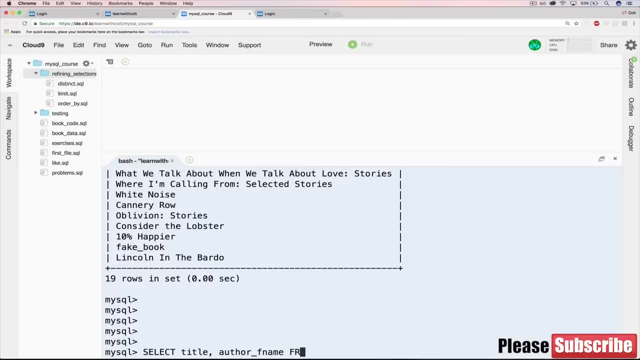 and author f name from books where, and then we'll do author f name like: and then this is where we need those wildcard symbols and we'll put da in between. so once again, this is saying anything followed by da, exactly da. so it can't be d and then s and then a. it has to be da and then anything. 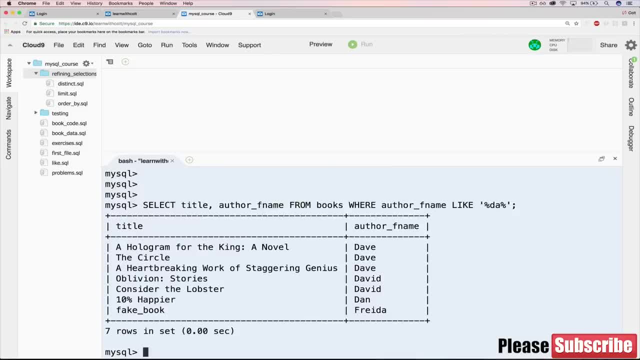 afterwards. so if I hit enter now, you'll see that it works. We get these authors: Dave, Dave, Dave, David, David, Dan and Frida, And you might notice, well, Frida, that doesn't start with DA, And you would. 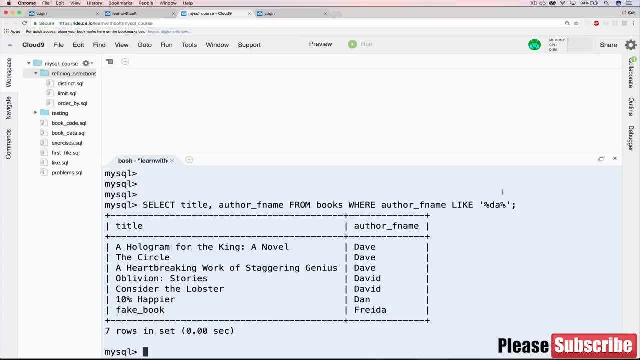 be right, It ends with DA, But it still meets this query's, or it still meets the conditions for this query, which is anything, DA, anything. So in this case it's F-R-E-I-D or F-R-E-I. 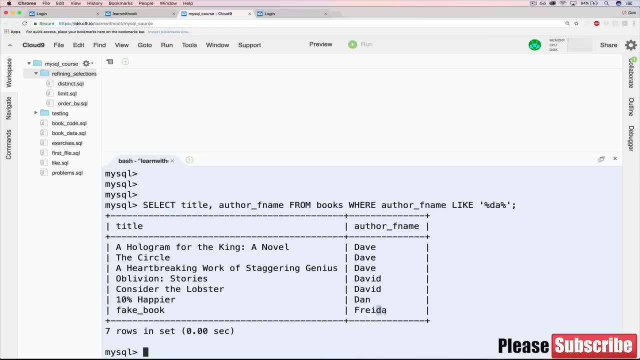 is meeting this, And then we have DA And then this wildcard. there's nothing afterwards, And that's perfectly fine. This is not saying there has to be something after the D and the A or something before. As you can see, we're matching DA- V-E, So there's nothing before it. 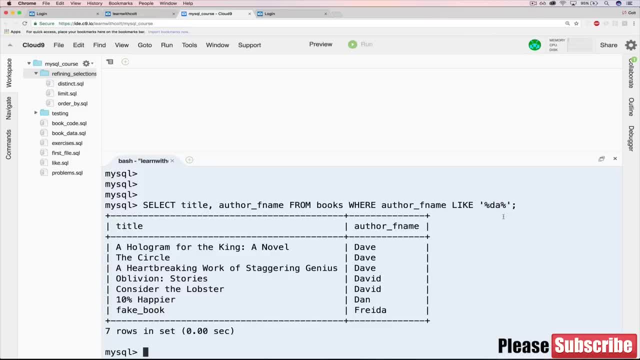 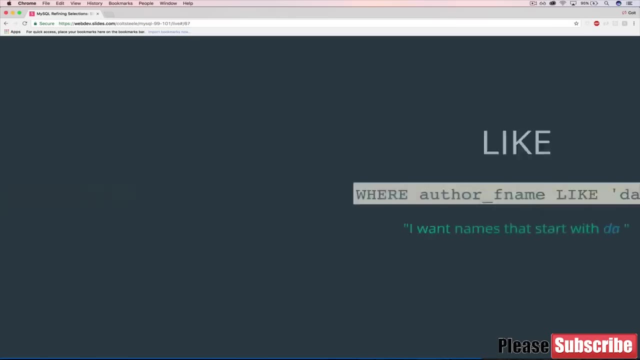 That's fine, Then DA And then V-E afterwards. So basically, this is all about pattern matching, And if we wanted to refine this so that we only get author first names that start exactly with Dave- or sorry, exactly with DA- we can do it like this: All we do is leave off that first wildcard. 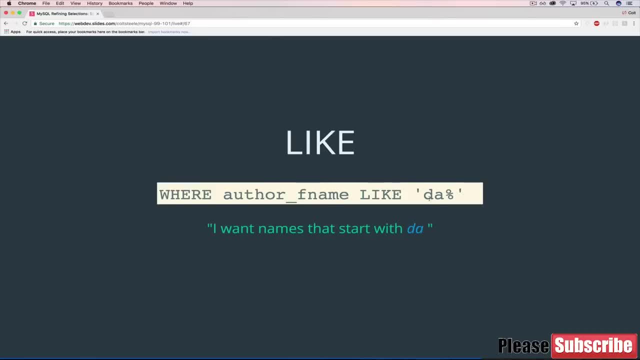 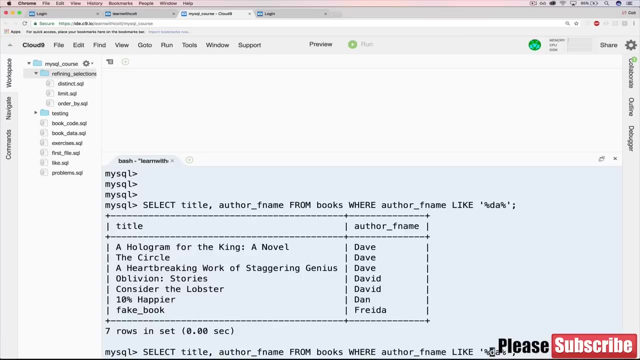 that first percentage sign And that says: I want to find author first names where they start with DA and then anything afterwards, So it could be Dana, David, Dave, Dan, Darwin, whatever. So if we just make that one small change and we delete that, 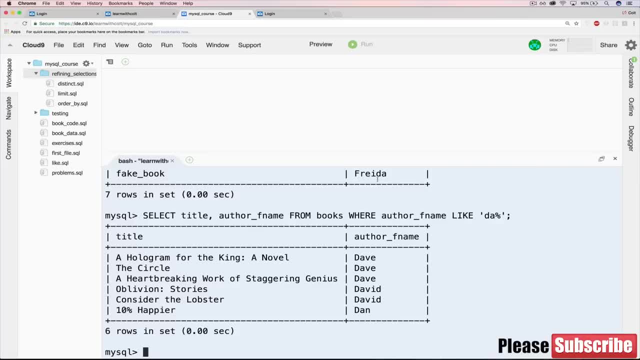 percentage sign. you can see Frida is gone. I'm sorry, Frida, Because Frida no longer fits the pattern that we're matching. Also, it's important to note that it is case insensitive. as you can see, This is lowercase d and a and it still matches all these uppercase d's and lowercase a's. 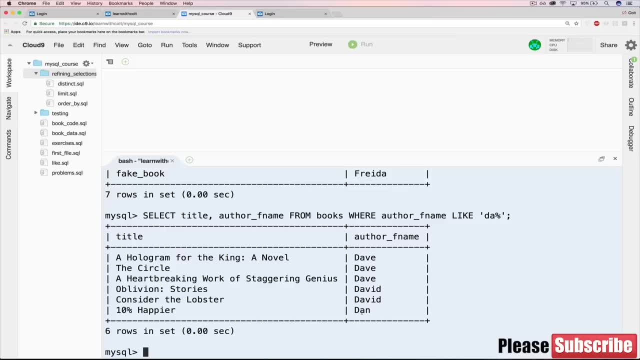 So if I wanted to do something slightly different, let's say, search all books where the title has the word the somewhere in there. It's pretty simple: It's just a select title from books where title like, and if I just say the, that's only going to give. 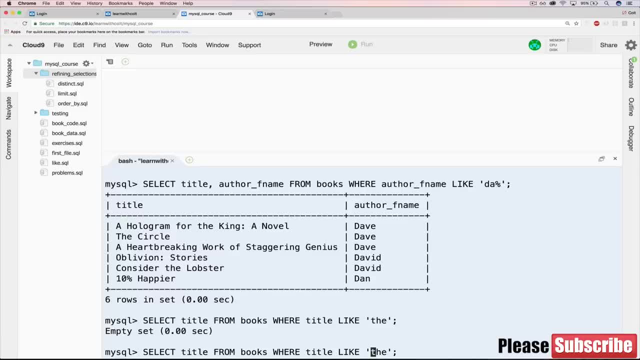 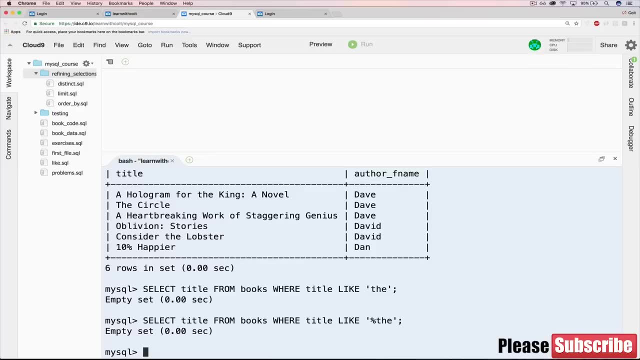 me books where it's exactly the and that's not what we want. So we want something followed by the And if we just leave it like this, that's not going to give us anything, because this, this is specifying. we want books where the title has anything and then ends with the letters T-H-E. 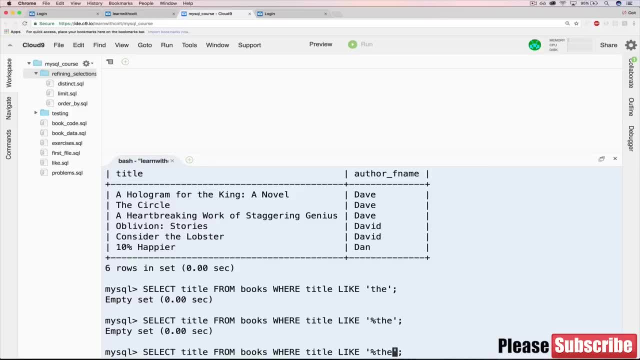 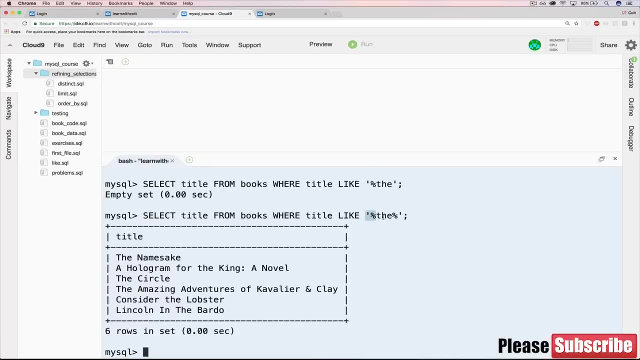 That's not really what we want. So we'll add another wildcard at the end And now that gives us all the books that have a title that has something, then T-H-E and then something else afterwards. So you can see, we get The Namesake A Hologram for the King, The Circle, The Amazing. 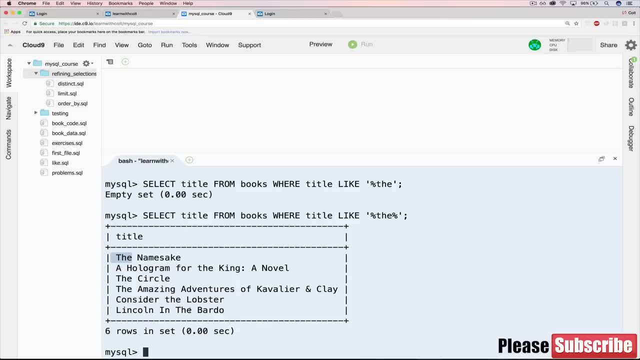 Adventures of Cavalier and Clay, Consider the Lobster and then Lincoln and the Bardo- Really good book. by the way, I know I've said that like 10 times It's a good book. So that's the basics of using like These percentage signs are very common. 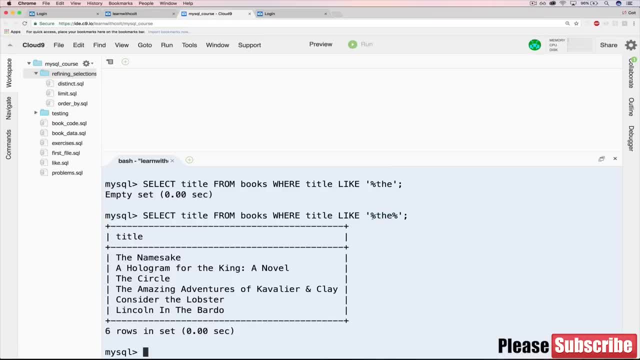 I know it looks kind of odd, but this is really really important. Think of when you're searching. I don't know you're on if you use Reddit, if you're ever searching for things on Reddit behind the scenes like is being employed, Or if you're searching on whatever site you search on. 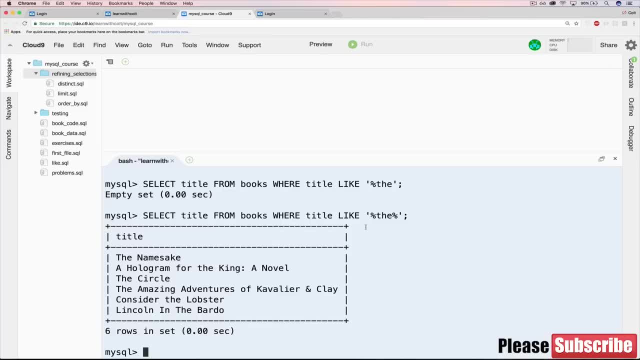 there's some form or variation of this, like going on where you're searching for things on Reddit and you're searching for things on LinkedIn. Whatever you search for, it's not being, it's not only matching exactly. So when I search for, 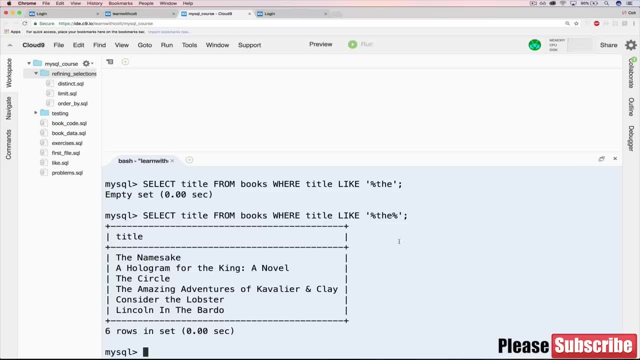 you know, on Amazon I type in: let's just go with my, let's say, Lord of the Rings. I search Lord of the Rings. It's not only going to give me books that have a title exactly of Lord of the Rings, It's going to give me books that have Lord of the Rings in the title somewhere. Obviously, 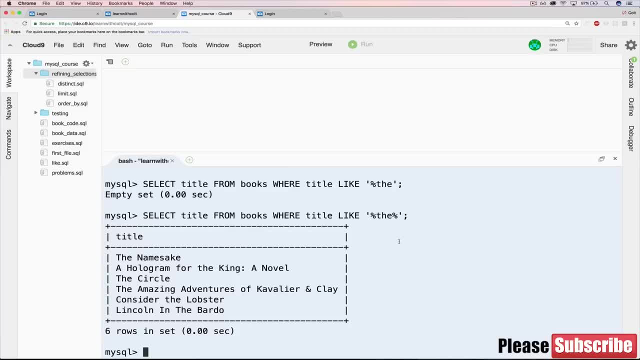 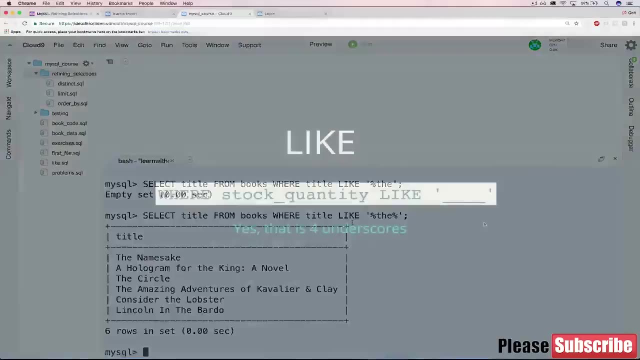 their search is much, much more complicated, where it also searches things, like you know, through comments and reviews and related books. There's this whole complicated graph network of how the search works, But the core idea, the simplest search that you could implement, uses like: So that's the basics, But there's 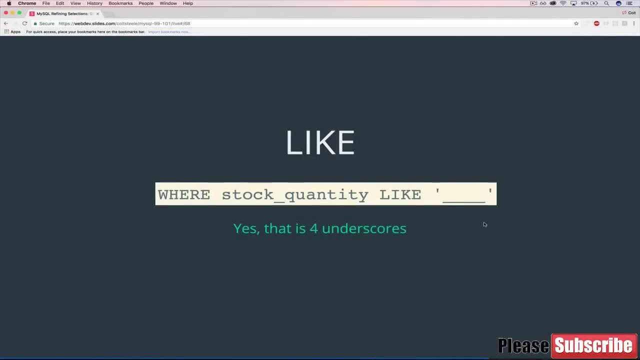 another wildcard character that I'll show you, which is the underscore. So here I have a really weird query. This is four underscores in a row. You'll just have to trust me that it's four, and it was hard to tell what this will do. So we're searching stock quantity, which is a number. 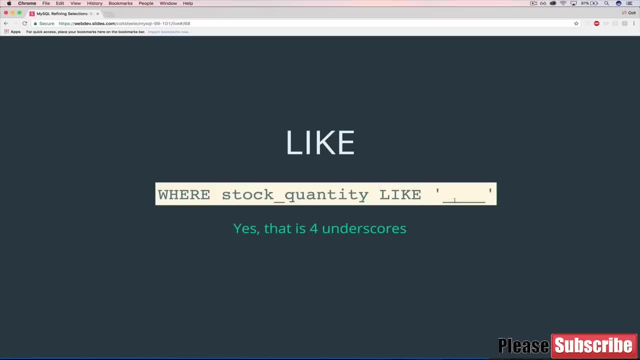 And we're trying to find where it's like four underscores And basically an underscore is a wildcard to specify exactly one character, any character, but exactly one. So four of them in a row is saying I want to find where the stock quantity is four characters long. So let me show. 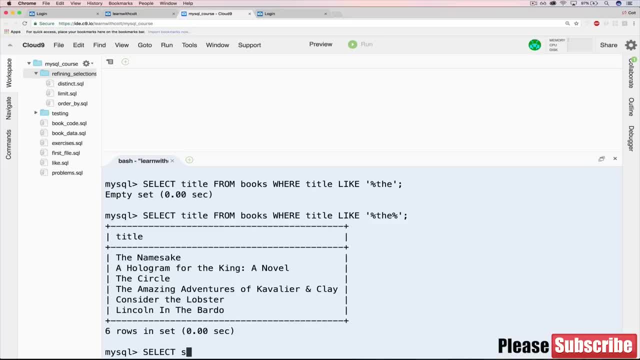 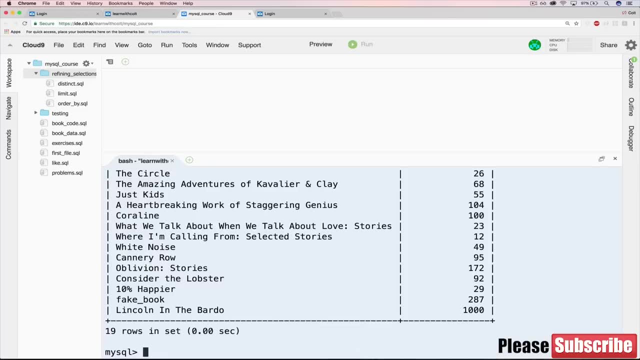 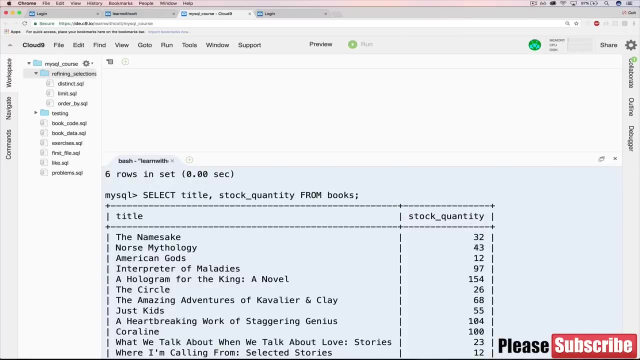 you why we might want to do that. If I do a select stock, let's do title and stock quantity from books, just like that You can see that we have stock quantity of two, or sorry, two digits. two digits: 32,, 43,, three. 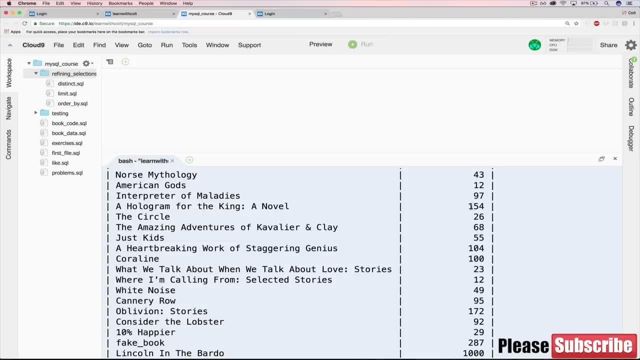 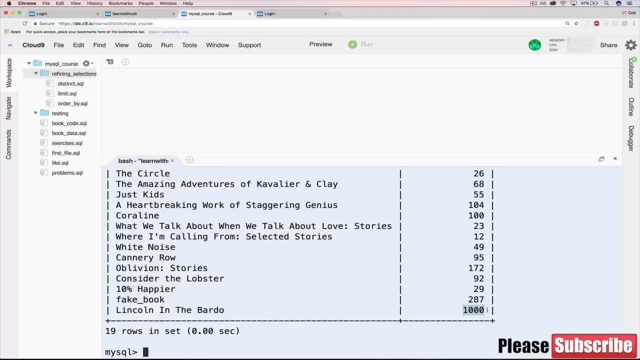 digits- Jeez, it's giving me a tough time- Digits 154.. And then this great book Linking in the Bardo has 1000 copies in stock. It's brand new. People don't know about it yet. They're not buying. 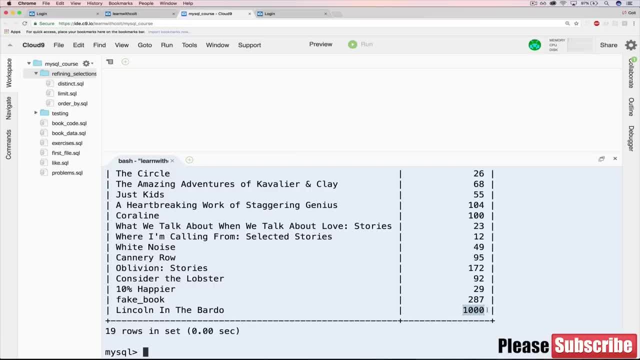 it. I'm sure people will buy it soon though, Once, of course, they realize what a great book it is. So if I wanted to select books where stock quantity is four digits long, I could use that wildcard, So let me just show that again. So select title and. 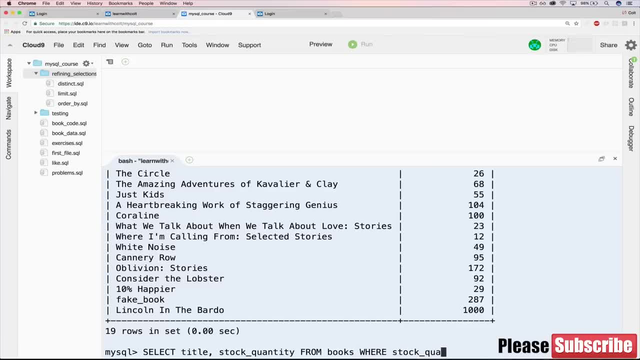 stock quantity from books where stock quantity like And all I have to do. so just to clarify: if I did this, that wildcard just means anything. So that's going to give us everything, And if I do four of them, it doesn't make a difference. That's not saying four characters, That's just four. 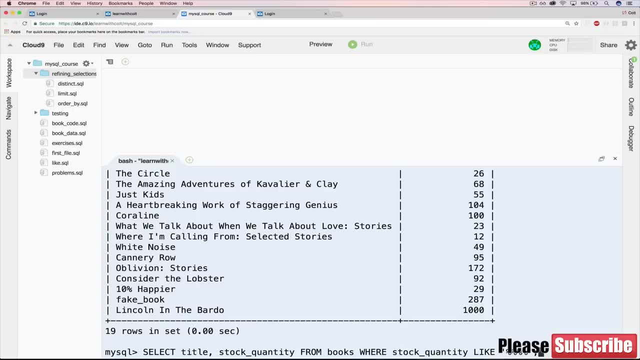 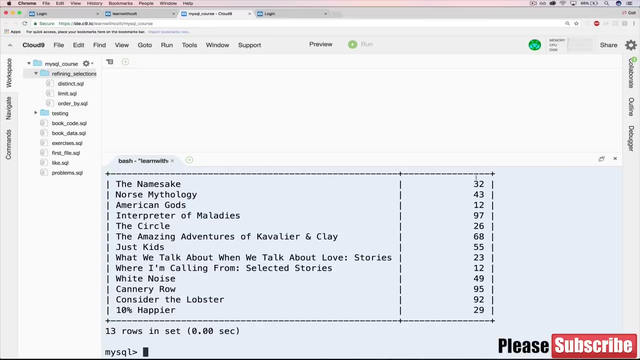 different ways of saying anything at all. It could be 1000 characters, It doesn't matter. So by adding underscores that's four. there you'll see, I get Linking in the Bardo. Or I could do two underscores And I only get the two-digit stock quantities. Now 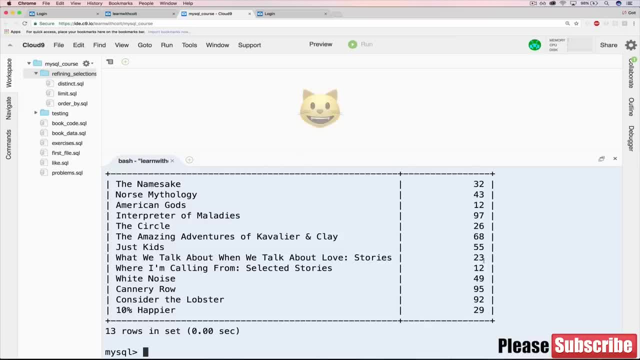 that's not to say the only time you use underscores is when you're trying: Yes, Blue, That's my cat. Are you going to say hi? She's now sitting on the computer. Ok, So back to where I was. Yeah. 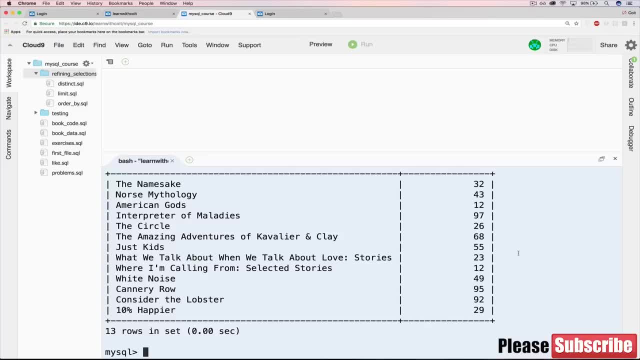 get this cat hair out of here. The underscore's not only used—and actually it's not even primarily used—for counting digits like that, but it's a way of specifying exactly one character. like I said, Let's say that we're working with phone numbers, And in the US they might. 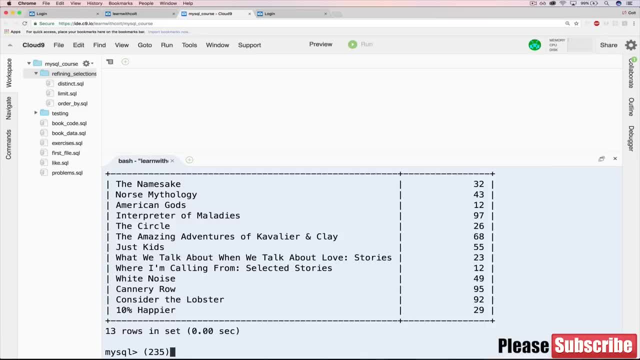 look something like this: So we have an area code in parentheses and then three digits, dash four digits, And if we wanted to match that pattern, we would have something like this: Okay, We would have something like this. We would have something like this: 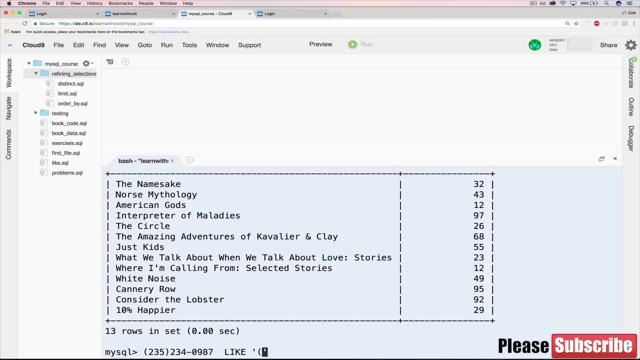 Okay, that looks like this, like: and we'd have our first parenthesis and if we just put this wild card there, that's going to say any number, any letters, whatever it is in between those parentheses. but we're actually looking for three digits and then another three digits after that parenthesis. 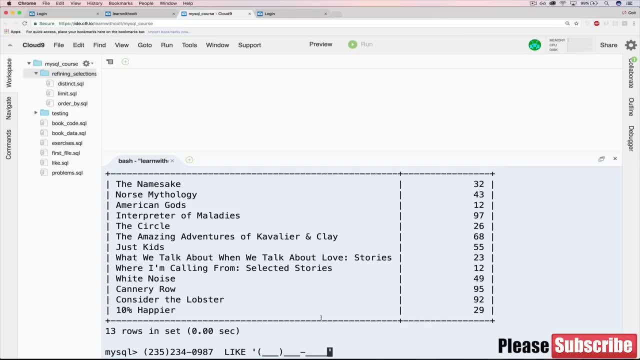 then a dash and then four digits. so basically we have these two wild cards at the end of the day, percent sign, which means anything or nothing, and then underscore, which is exactly one thing, and you can chain them together to match patterns. then that brings up another question, which is: but 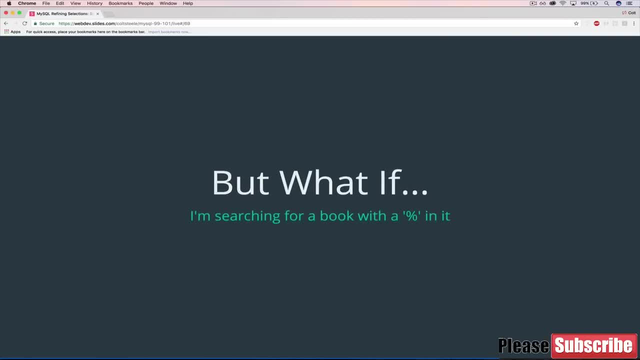 what if i'm searching for a book that has a percent sign in it? how would i do that? and you may have noticed that i expertly planted a book title with percent sign in it. i was thinking ahead for once. how would we select that? or there's also a book title that's not so creative, that has an underscore in it. 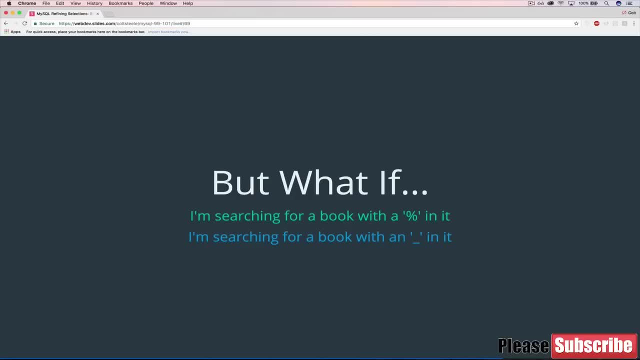 how would i select that one? if these characters are special wild card characters, how do i actually search for the, the exact character percent sign or the exact character underscore? and the answer is actually pretty straightforward. um, we use what's known as an escape character. in this case, i always forget which one's backwards and forward slash, but whichever, 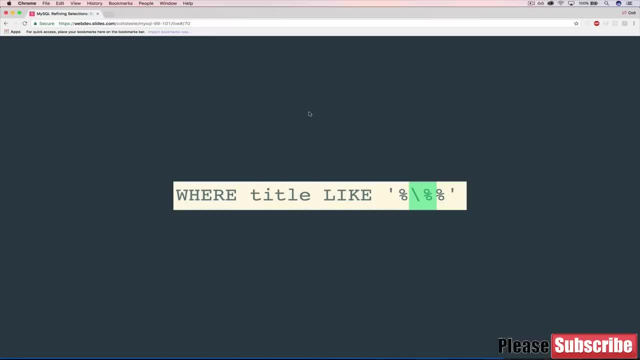 this is the one over the enter key. pretty sure that is backslash. so backslash percent sign is going to match a percent sign. so this entire thing right here is basically saying percent sign, likewise with underscores. backslash. underscore is the escape character, so let's put that into. 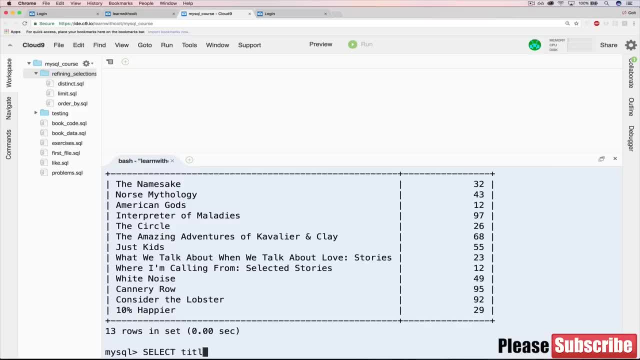 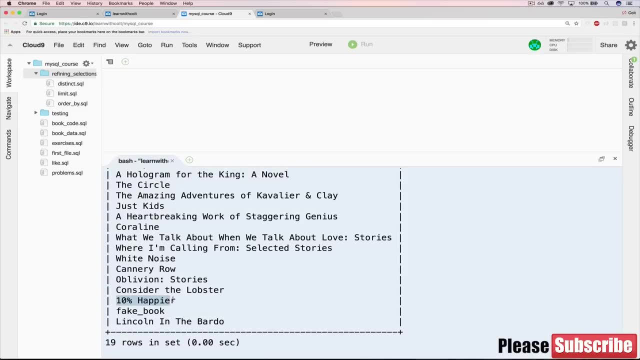 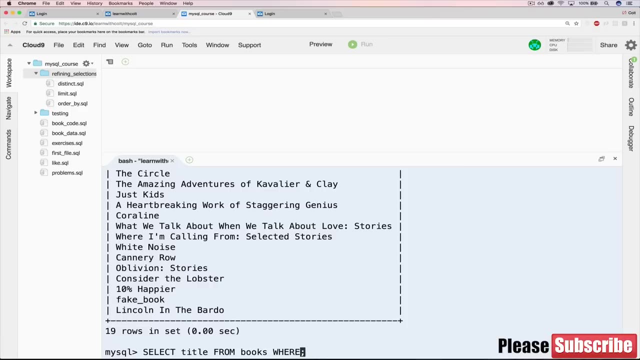 practice. let's try it out. so we'll select title from books and we'll just do that first of all, and then when we we go down saying myself we'll go to glossary, we've got like, and you'll see we've got 10 happier and then fake underscore book. so let's start with 10 happier. 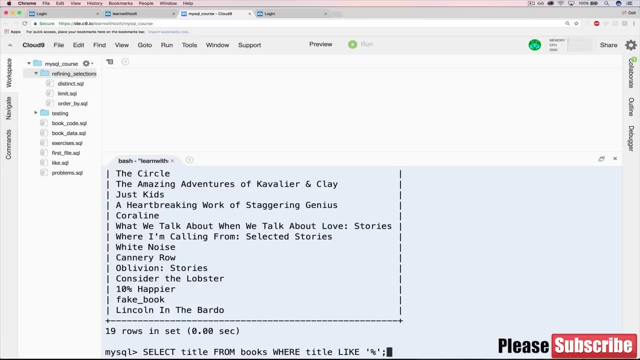 so i want to select title from book, from books where title like and just. i mean this should be clear by now. but if we tried to do this, that's not going to work, that's going to give us everything. but if i tried to say, okay, percent sign. 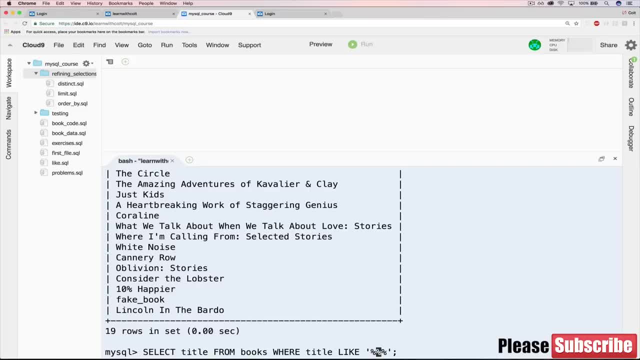 that means anything and then a percent sign and then anything afterwards. that's not going to work either, because that's basically just three different ways of saying anything and we just" at all in the title. so that's where we need our backslash. and now what you could read this as: 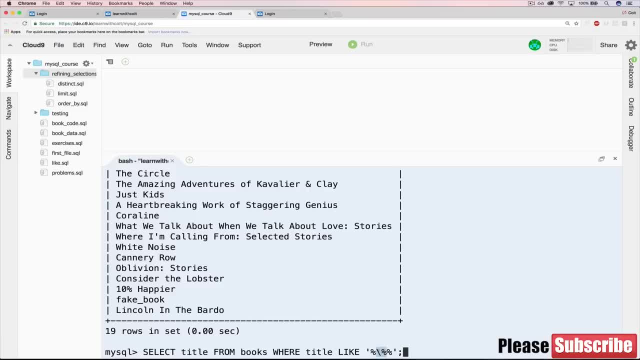 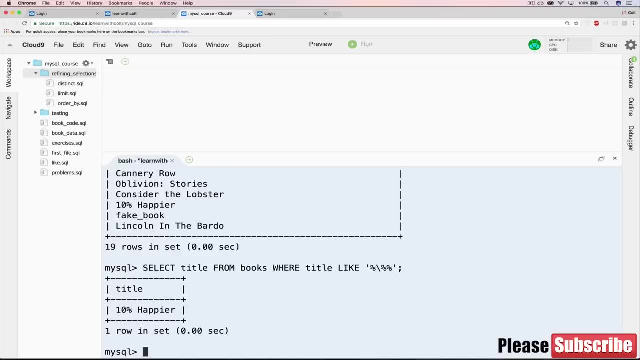 you could condense this to say: exactly a percent, sign one percentage, sign anything before, anything after, and there we go. that's how we get 10. happier same thing with the underscore. i won't go through that whole routine again. we just replace that backslash percent with backslash underscore. 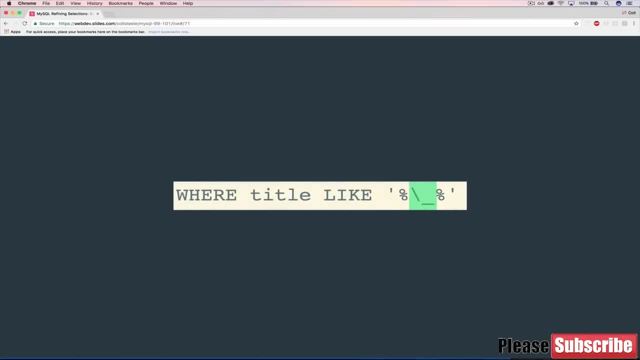 and that gives us fake book. all right. so that's all that there is to like for now. it's very, very useful. we'll be using it quite a bit in this course. it's probably one of the most commonly used things in mysql or in sql when doing queries. in all likelihood you won't be matching percent. 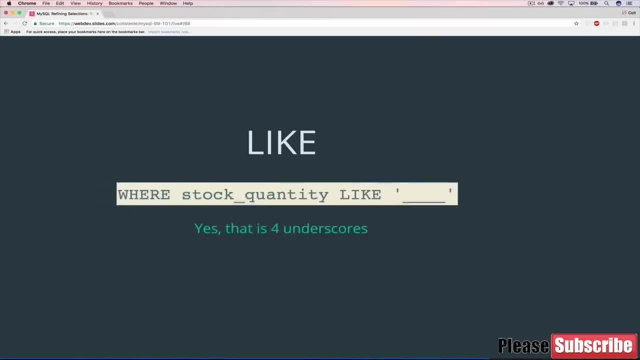 signs or underscores all that often. but you'll be doing things like this all the time, where you're using the percent wildcard and the underscore wildcard to match patterns. okay, next up exercises: ohidoki, heart of choki. yep, that's how i'm starting this video off. uh, it's your turn, so. 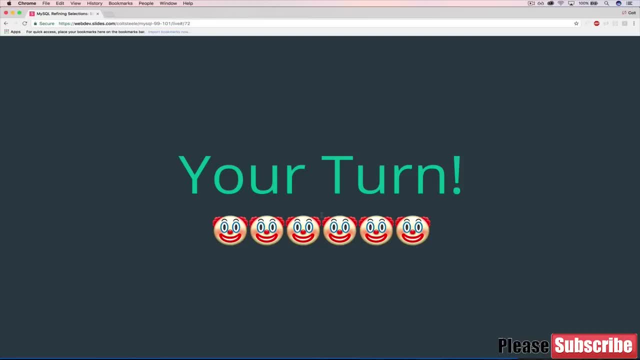 we've covered four different things here, four new tools for this mysterious, magical toolbox. we've got distinct as well as order by, and then limit, and then finally like, and you're going to put those to use along with some of the stuff you've learned up until this point, with a couple. 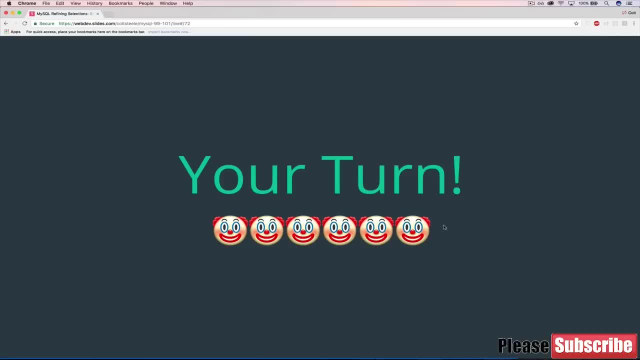 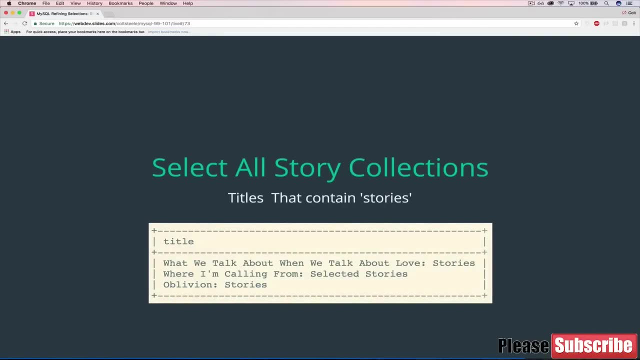 of exercises, and there are some clown emojis here to show you how excited you should be, and they're not at all creepy. so here's the first thing i need you to do, or i'd like you to do: please, please, do it: select all story collections. so some of these books have titles that contain the word stories, which tells. 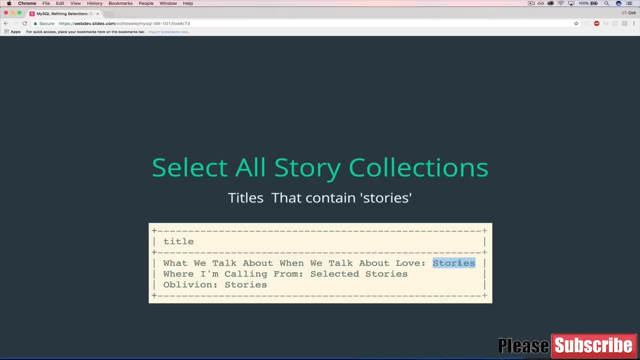 you that they're a collection of stories. what we talk about when we talk about love stories- really good read, by the way- where i'm calling from selected stories, oblivion stories. so, using what we just saw, and that's something i just want to point out- for all of these exercises, there are ways that 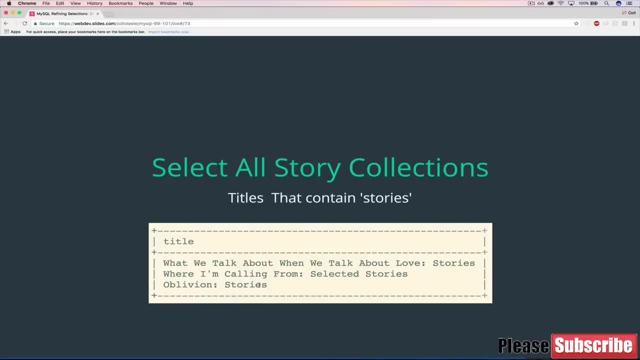 you could directly select things, maybe a little bit easier, or you could cheat in a way, but make sure that you do it the way that i specify, please, using the things you just learned, so specifically: titles that contain the word stories- not exactly stories, but something that contains stories in it. 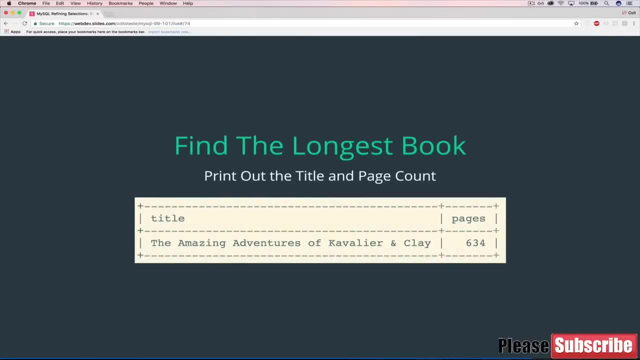 so that's the first one, all right, and then the next one. find the longest book in the entire database or in the entire books table. so this is what you should get back. print out the title and the pages. the amazing adventures of cavalier and clay is 634 pages. 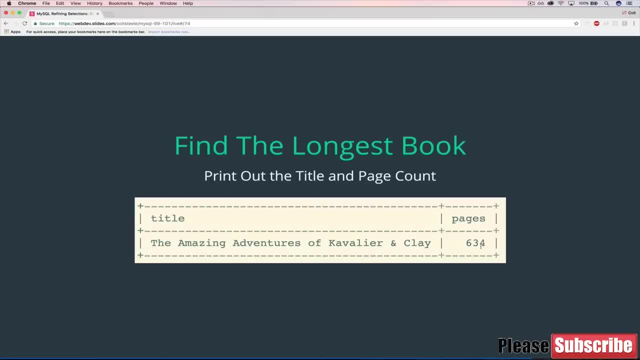 of course, don't just select based off of where pages is exactly 634 or where the title is the amazing adventures of cavalier and clay. please do it the right way, so that your query would always work, no matter how many books are in the table and what they're named and how many pages they they. 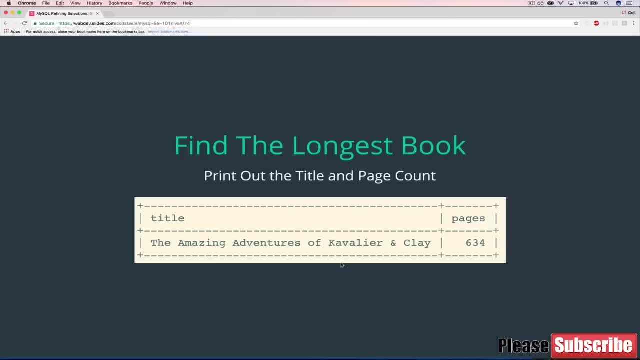 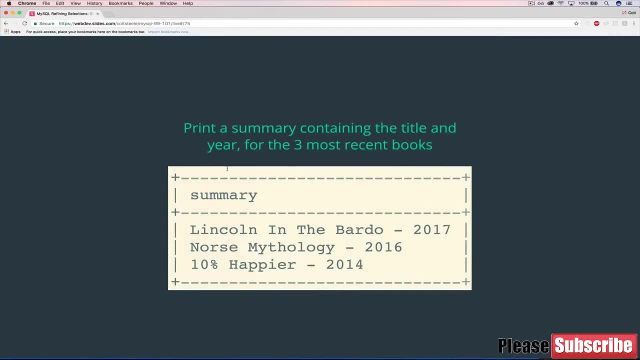 have, it will always get the longest book. okay, then the next problem: print a summary. in our case, a summary contains the title, dash the year and print three, only three, of the most recent books, so 2017, 2016 and 2014.. so again a summary, and it says up here: it says summary, so that remember how to do that- the title. 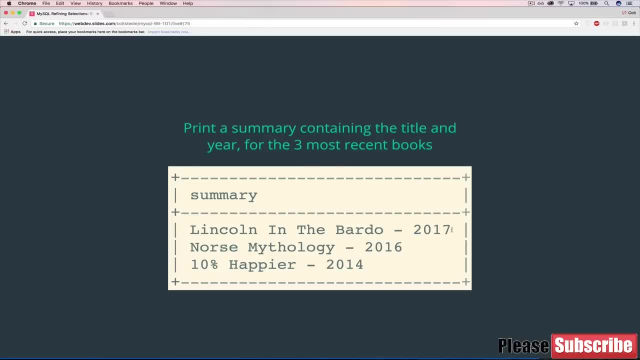 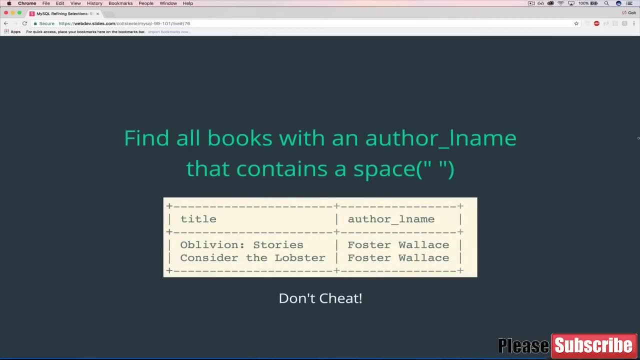 dash the year it was released, and then only print out the first chapter and then another chapter and then the study. it would be the three most recently released books. all right. next next up is find all the books whose author's last name contains a space character, and it's only david foster wallace in our case. don't cheat and just say: 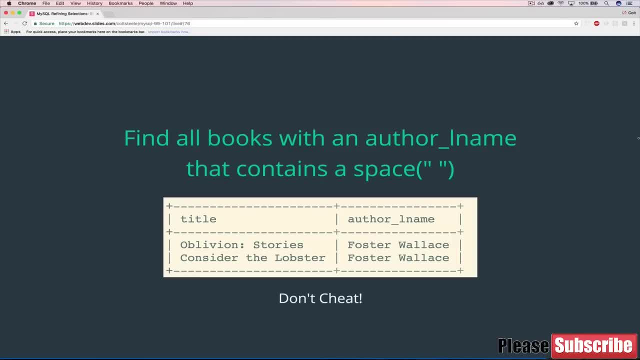 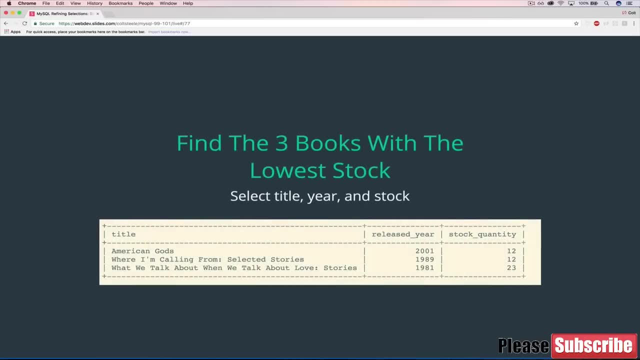 where author l name is exactly foster space wallace. but how can you find any author last name that has a space in it? and then, once you do that number in stock, the lowest stock quantity- so as you can see here we've got American Gods- is 12. where I'm calling from has 12. what we talked about. 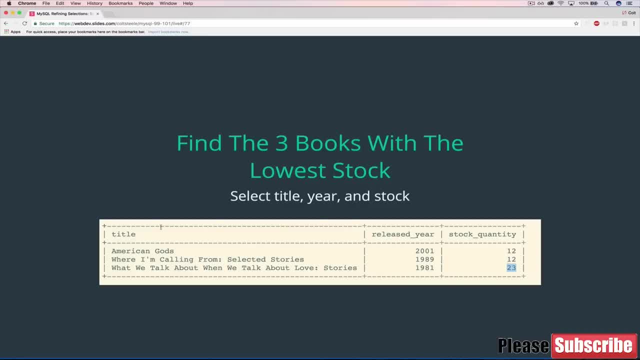 when we talk about love, has 23 and I'd like you to print the title, the release year and the stock quantity, so just to reiterate, the three lowest stocks. all right, then we have this one: print the title and the author last name. so you've. 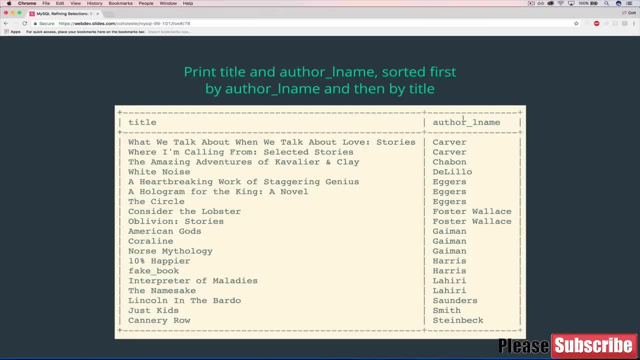 got title author, I'll name sorted by the author's last name. so this is all of the books, by the way. so sort by the author last name and then sort by title, because some of these authors, for example Carver or Eggers or Gaiman, have 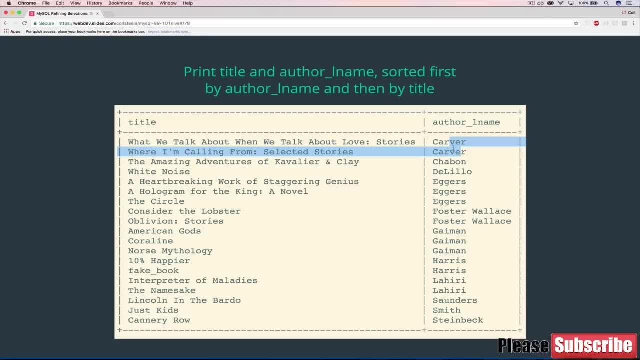 multiple books. so if we look at Carver, for instance, Carver has what we talked about, blah, blah, blah. where I'm calling from, what we talked about comes before where I'm calling from, alphabetically, if that makes sense. same thing with Eggers: a heartbreaking, a hologram, the circle. so sort first by the last name of the author and then on. 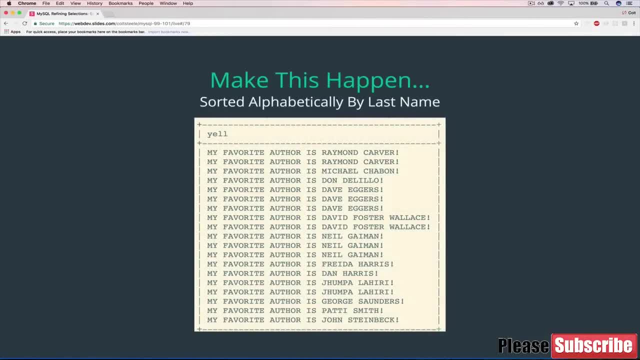 top of that, the title. then we've got this one. just make this happen. it's kind of difficult to write out exactly what's happening. the main idea is that we're going to go through every book. you're gonna print out this string here. my favorite author is- and this is yelling in all caps- I won't wake my neighbors. 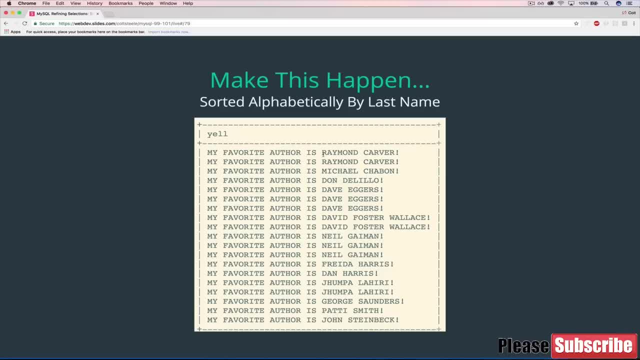 it's kind of late, but my favorite author is, and then the author's first name capitalized is, and the author's last name capitalized, and an exclamation point at the end, and do that for every book sorted alphabetically by the author's last name, so you can see Carver comes first, Eggers, Foster, Wallace, Gaiman, down to Steinbeck. 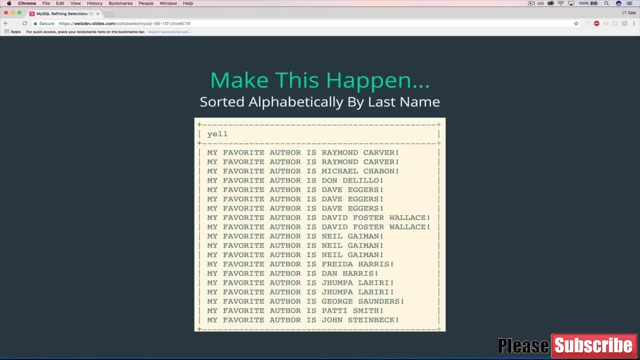 and then make sure you call it. yell up here. yes, it's a bit of a complicated one, but fortunately it's last. hopefully you can make this one work. it's a little bit long. good luck. see you in the solution video. all right, so hopefully you made it. 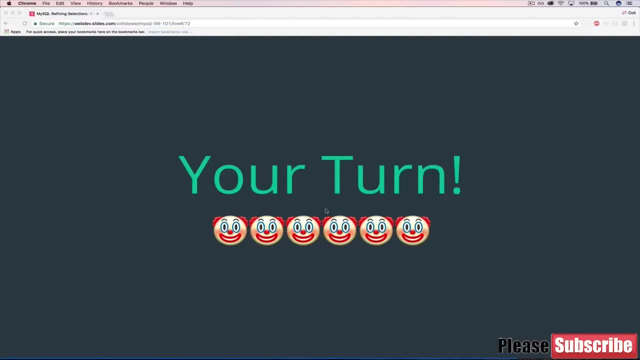 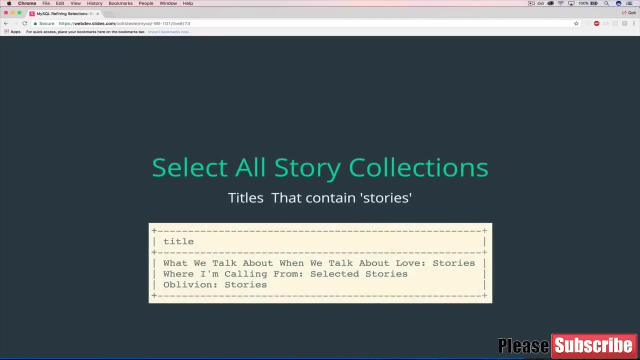 through those exercises, or maybe you're just wanting to watch the solutions, or maybe you're here accidentally. however, you got here. what I'm gonna do in this video is go over the solutions to the previous video, and that's a bad noise. why'd that happen? all right, so the first one: select all story collections that so. 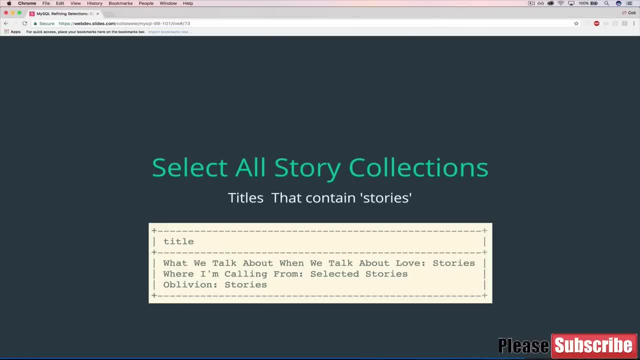 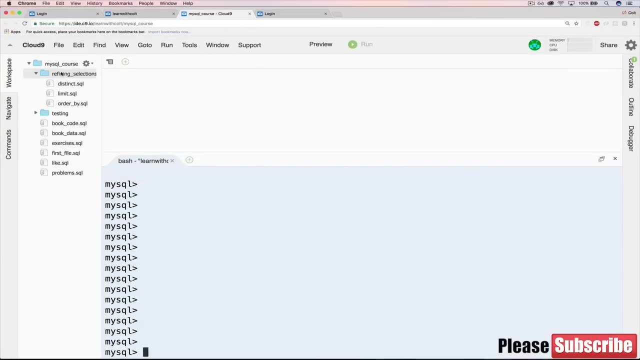 there's our titles that contain the word stories in them somewhere and we just want to print the title. so I'm going to go over here and make some space, and the first thing that I'll do is just make a new file and I'll just call it exercises dot SQL, and then I'll open that up and we'll start off with. 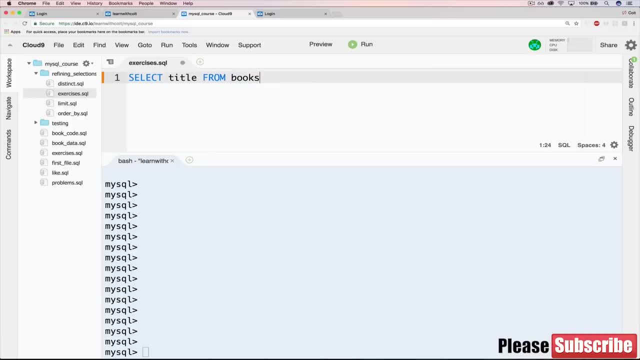 this first one: select title from books, and we'll start there. just make sure we're doing everything correctly: source refining, selections, slash exercises, dot SQL. make sure that, okay, it's working. selecting the titles: so now we only want the ones that contain stories. so that's going to be aware and we're gonna do title like: and this is: 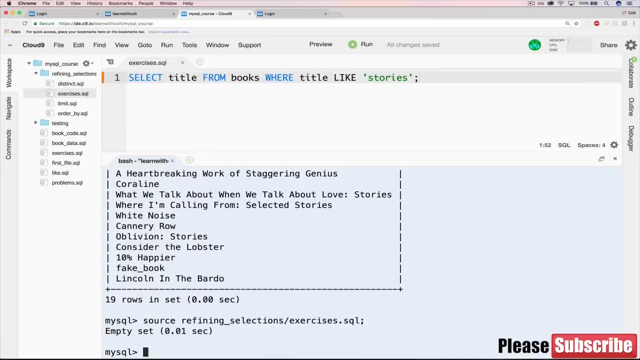 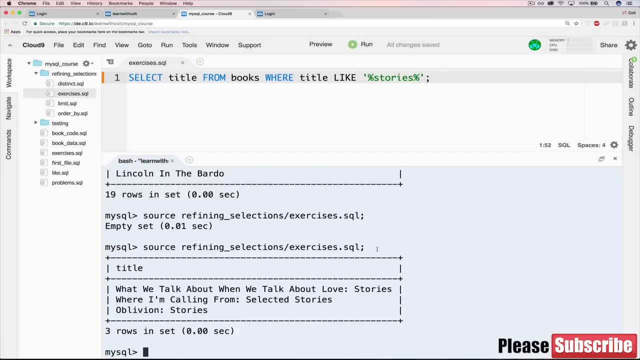 you know, if we just do stories, it's not gonna work. that gives us exactly stories. we're going to want that wildcard character, just like that, and now we get what we're looking for technically with our specific data. we could leave that last percentage sign up and then we're going to go over here and we're going to 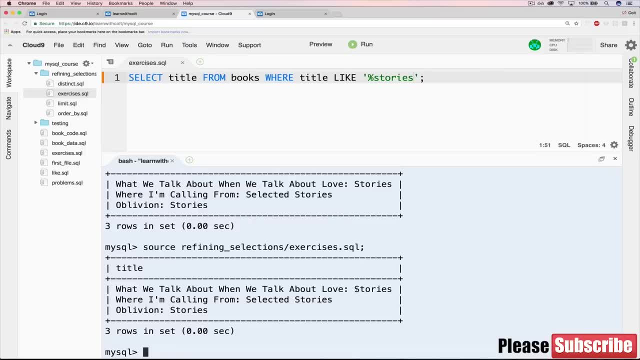 take that last percentage, sign off that last wildcard, because all of the books that contain the word stories it comes at the end, but that may not always be the case. there might be a book out there called my favorite stories for kids, something like that, and if we wanted this truly to just find all books that. 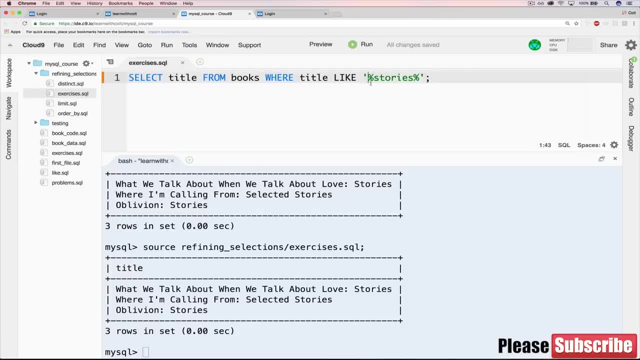 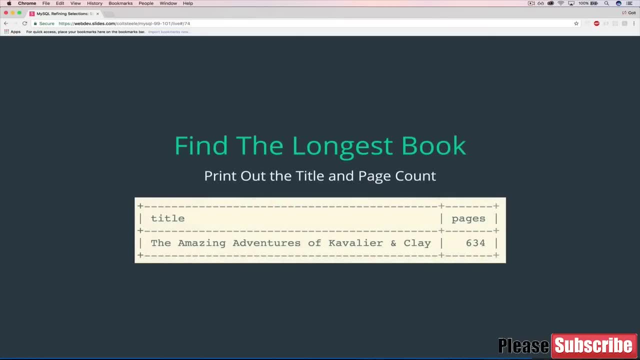 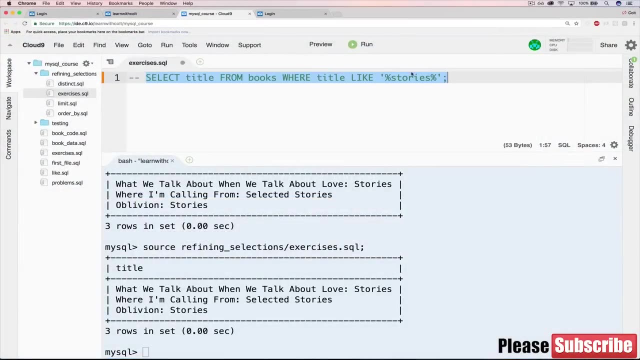 have stories in the title. we need both of those wildcard characters. all right, so that's the first one. next up, find the longest book. so print out the title and the page count for the the one longest book. so we'll go ahead and comment this line out and let's just do a select title and pages from books, just. 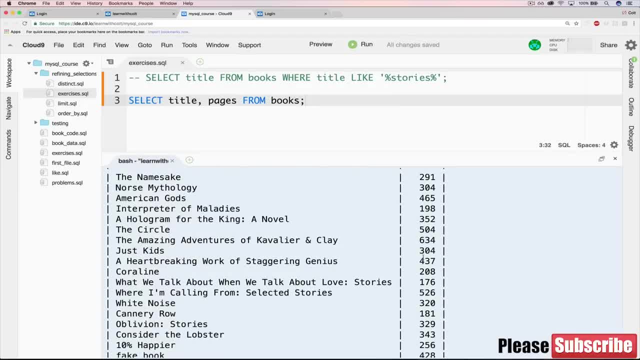 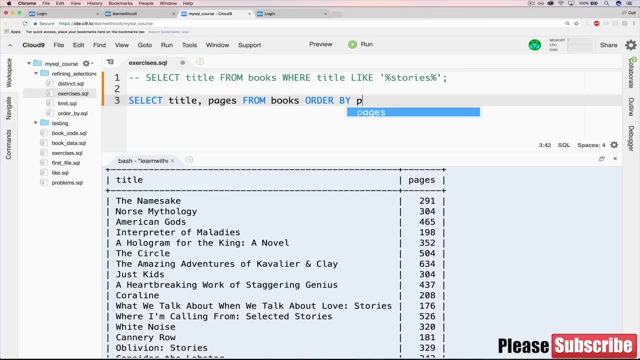 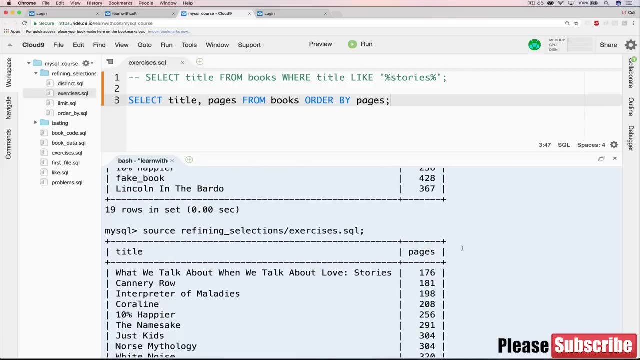 like that to start. okay, so now what we want to do is sort them. we'll sort them by the pages. so that's an order by pages, and if we just do the default sort, remember that we get ascending rather than descending, which is what we want. what we're going to do is use limit to give us the first result. but right now, 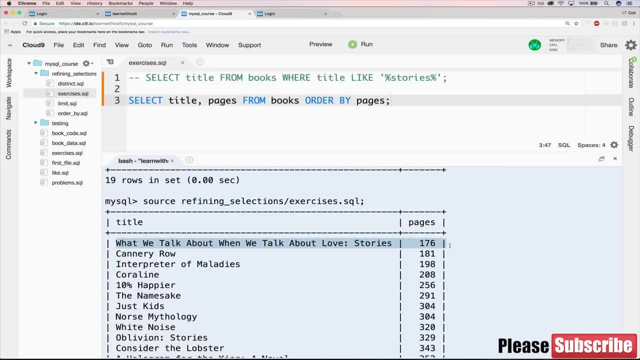 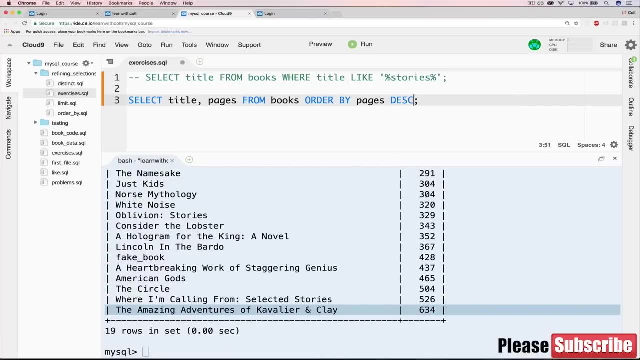 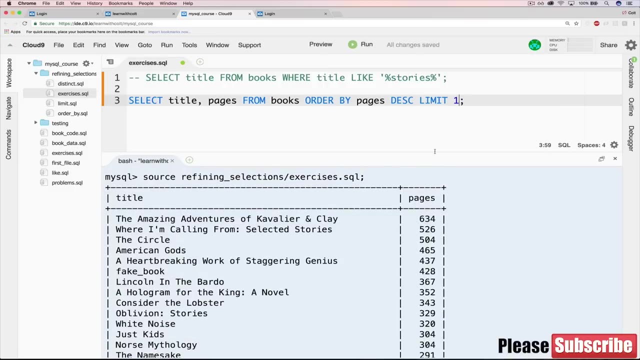 if we do limit one, it's going to give us the shortest book rather than the longest one. so we want to reverse that sort with the descending order. so now the first one is the longest and then we just add our limit one and we run it again and again, and again. 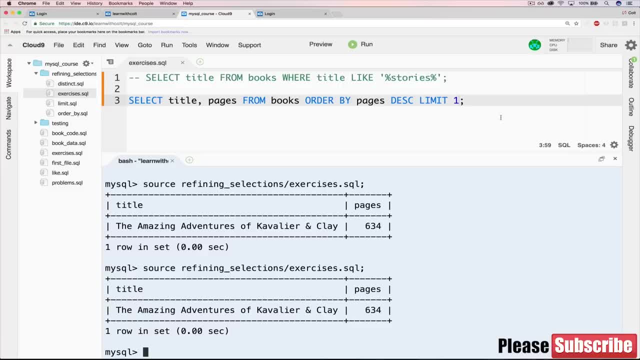 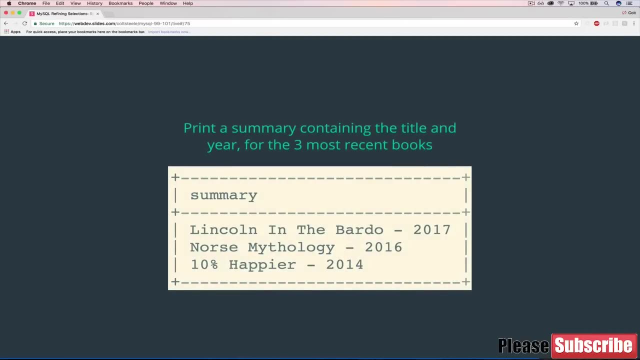 and it always works. and so whatever book has the longest page count will always be what is printed out here. all right, so that's that one. let's comment it out and move on. print out a summary containing the title and year for the three most recent books. so this one required you to not only use order by and limit or 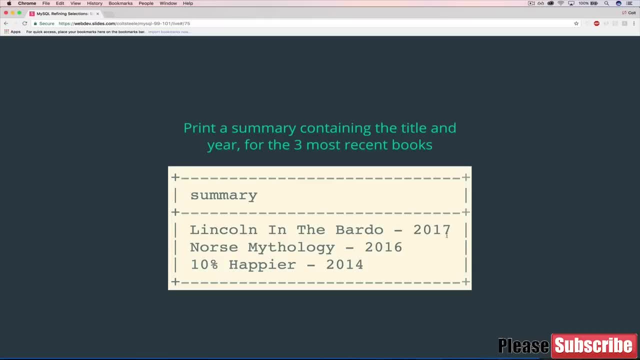 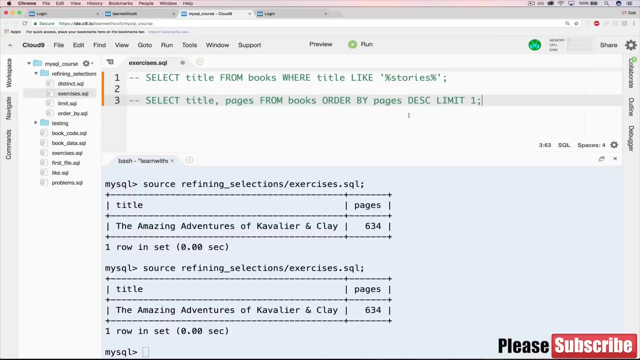 ordering by most recent year and then limiting to three, but you also needed to use order by and limit, so that's the one that we're going to use for this one. so concatenate to concatenate the title with a dash with a year, so let's do that. 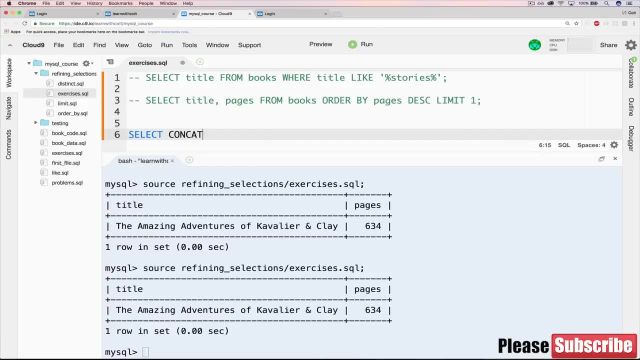 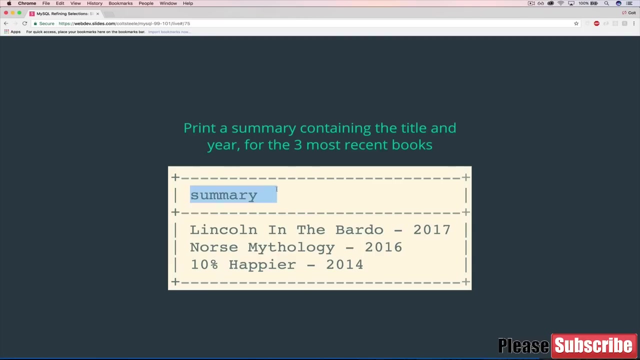 now let's just start by doing this: select concat and it was title comma. then we have a space and a dash and a space comma released here and we'll start with just that from books save. okay, oh, the other thing we wanted to do is clean this up. so it says summary up there. so this is also review. we'll say: 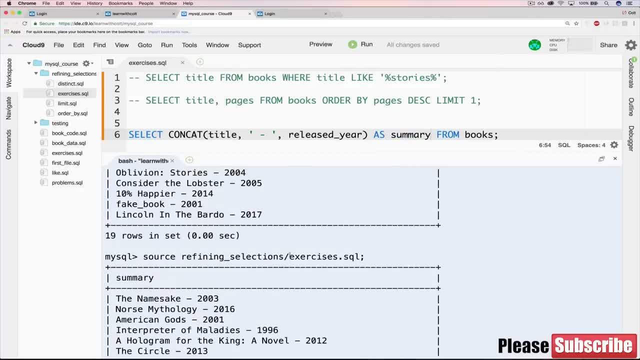 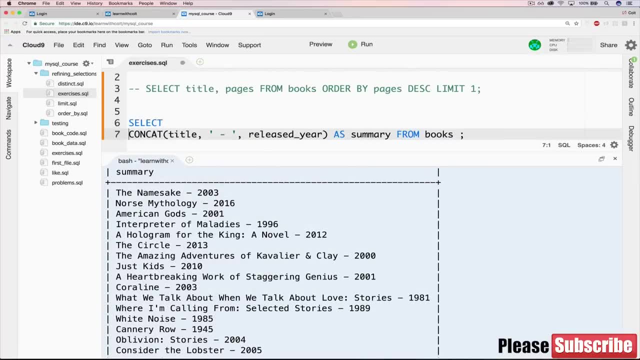 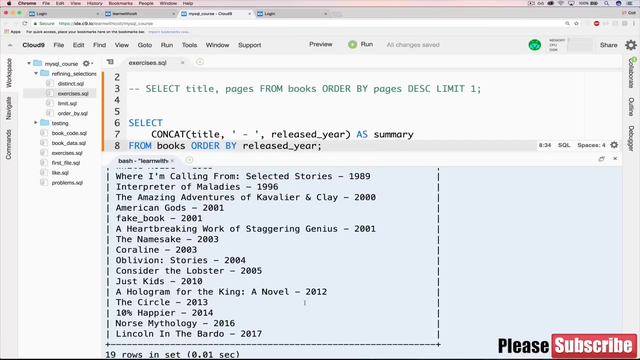 as summary. okay, so now we get that. now we want to order them by most recent and let's break this up onto some different lines here from books: order by, and we'll order by, released here. and if we try that, now we also see that we have a summary and we want to order by release here and we 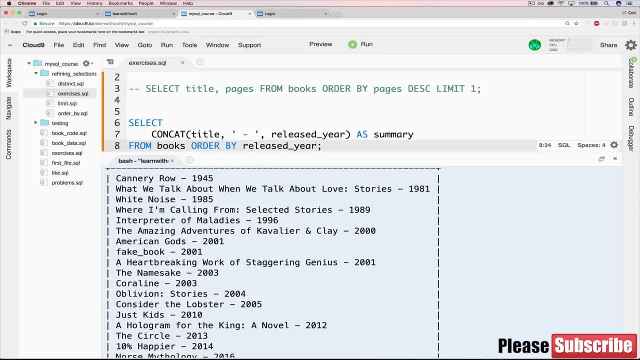 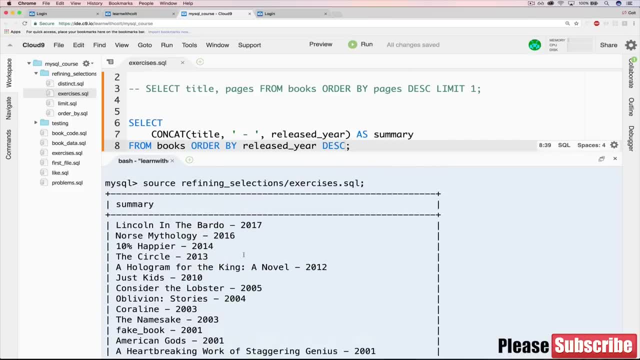 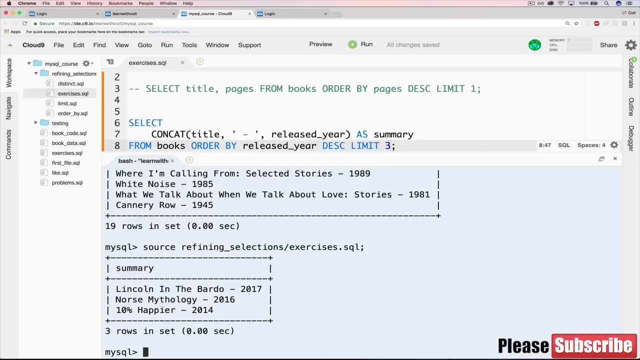 see that it does work. but it's in the opposite order that we want. we want most recent, so we need to reverse that again with descending, and then finally, we want to limit it to the first three. limit three, or, if you want to get fancy, we could do this, but I don't like doing that. so that's much easier, okay, that. 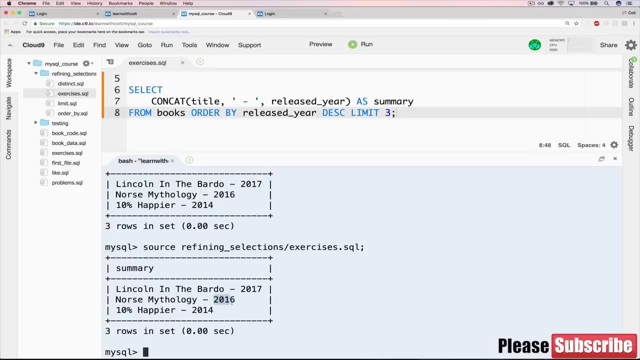 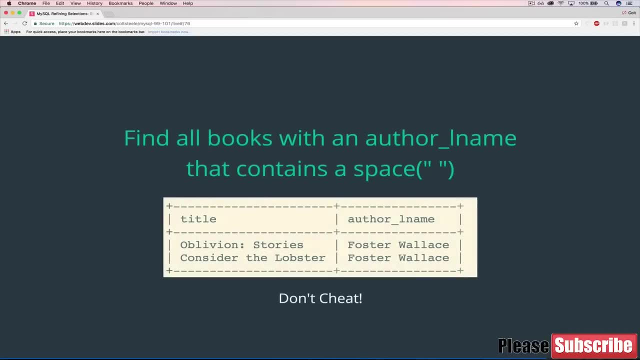 gives us Lincoln and the Bardo. dash 2017. Norse mythology. dash 20: 10% happier. dash 2014. summary: that's all good. to go next up: find all the books that have an author last name containing a space, and don't cheat by just doing. 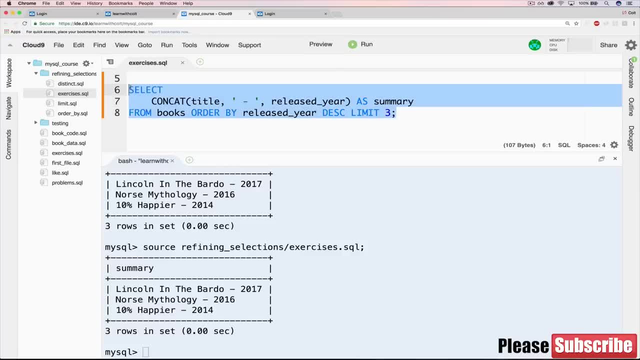 Foster Wallace. so let's comment this out first. this one's actually pretty short and easy. it's just a select and we're looking for a title and author l-name, select title comma author l-name where author l-name like- and of course we can't just say space, because that's only gonna find authors whose last name is. 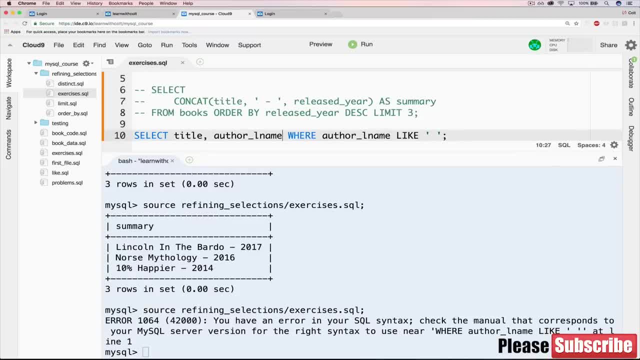 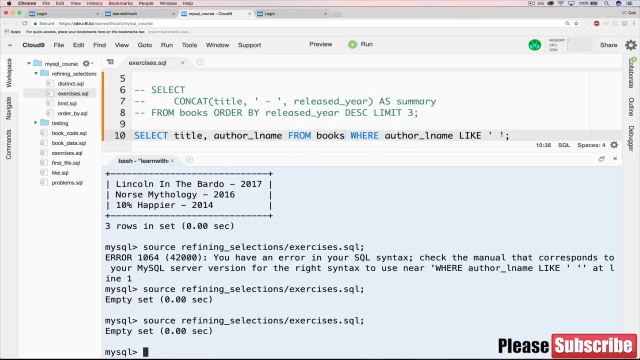 exactly space and it looks like- oh, I'm forgetting from books. hopefully you caught that before I did. but back to what I was saying: this isn't gonna work because we don't have any authors whose last name is space. so what we want is that wild card on either side, anything with a space and 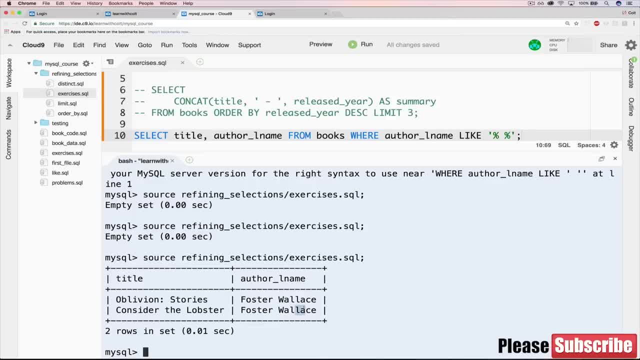 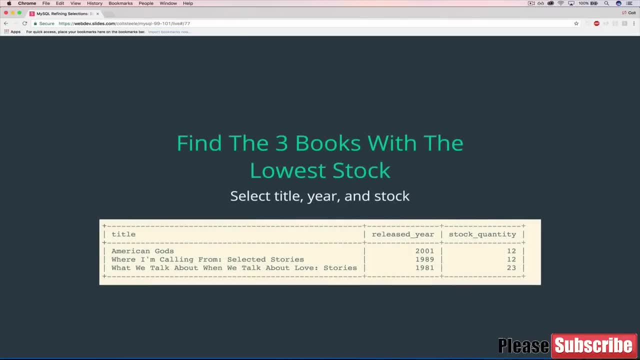 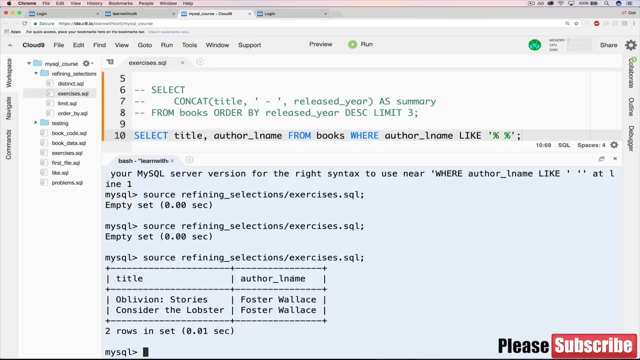 then anything afterwards. now we get Foster Wallace and that's it for that one. next up, find three books with the lowest stock. so we want the title, the release year and the stock quantity: three books with the lowest stock. so let's start with commenting this out, just like we've done. 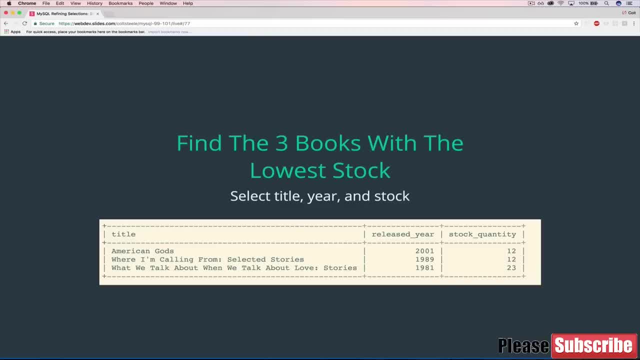 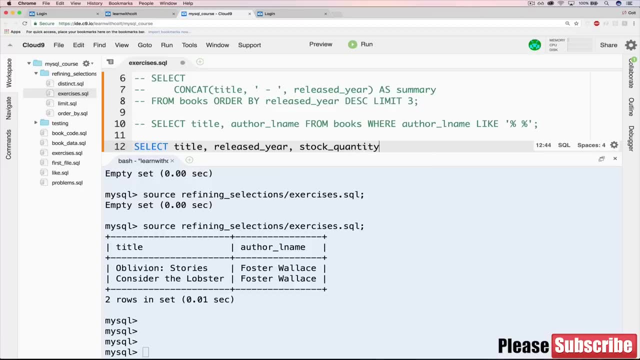 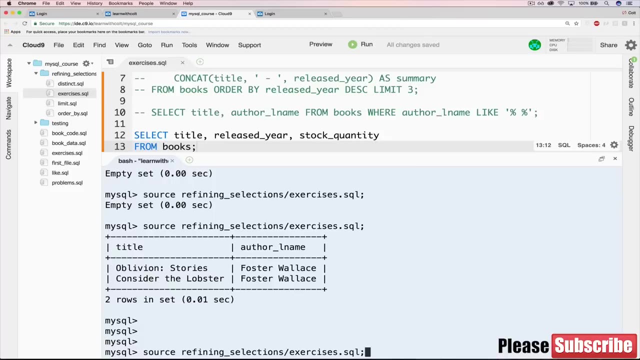 with all of these studies- this is the first one. we're checking out the book. the others Select title, What else was it? Released year and stock quantity. Okay, Just like that, And we'll have our from books. We'll start there. Make sure that works, Okay. So now what we want to do is sort them by stock. 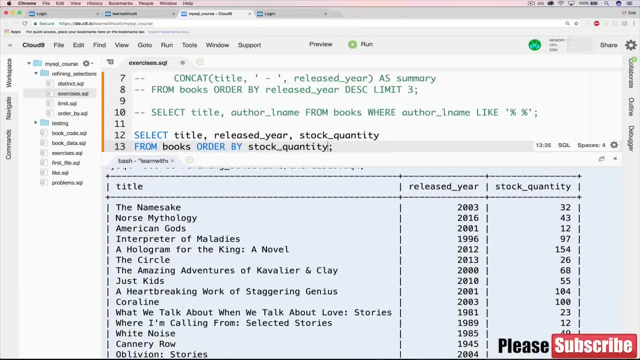 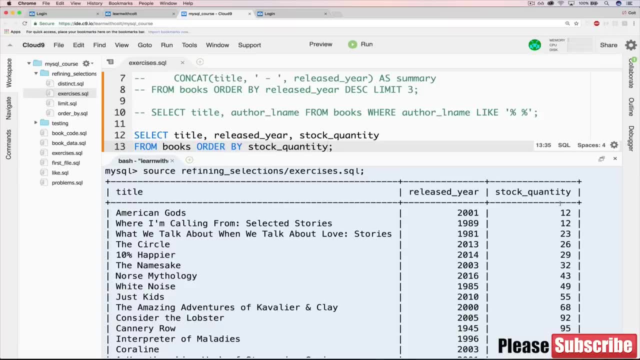 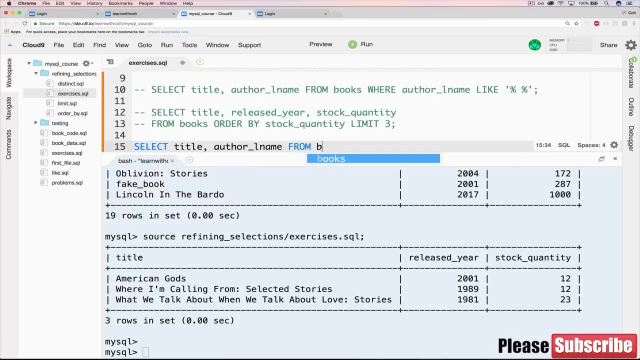 quantity. So that's just an order by stock quantity And you can see that gives us the order we want. We want them to be in ascending order this time rather than descending, because we're looking for the lowest stock quantity- 12- all the way up to 1,000.. Okay, And then we want: 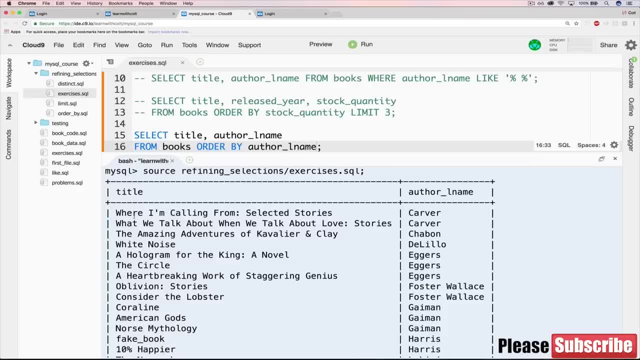 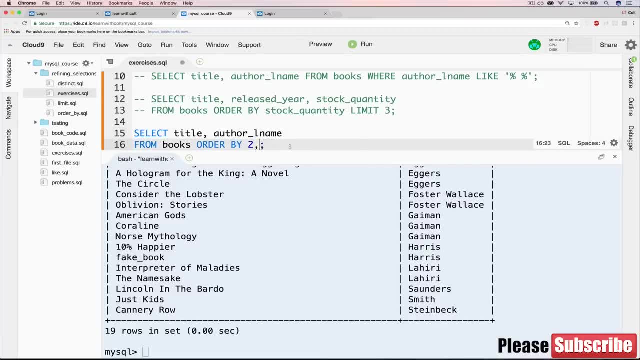 to limit it to three. I don't know why I picked three so many times in these exercises. Let's try it now with that limit three And there we go. American gods, where I'm calling from what we talk about when we talk about love, That's what we're looking for. 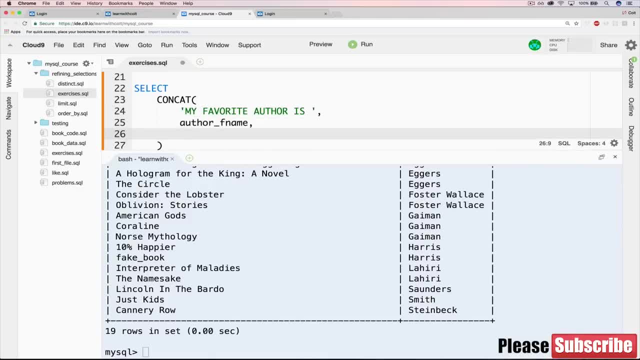 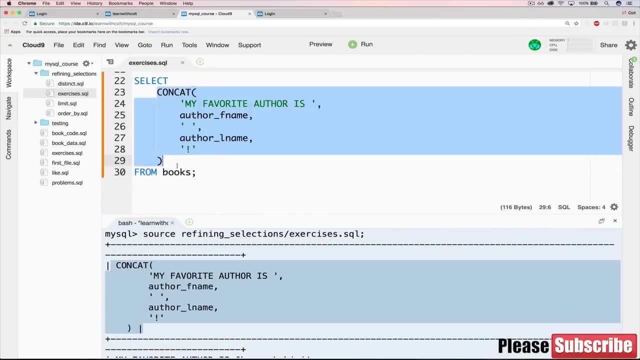 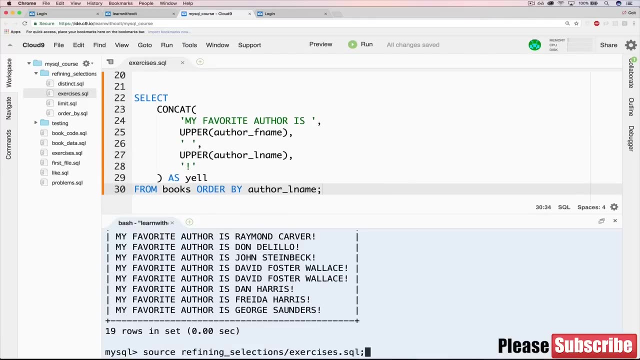 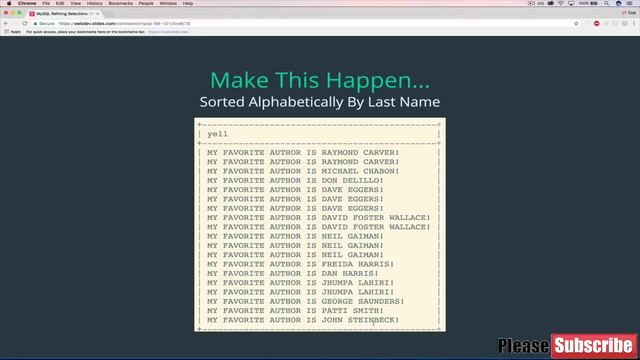 Then we've got this one: Print the title and author last name, sorted first by author last name and then by title. So let's get the title and author last name to print first. Select title, author L name from books, Just like that, And at this point we all know what that does. 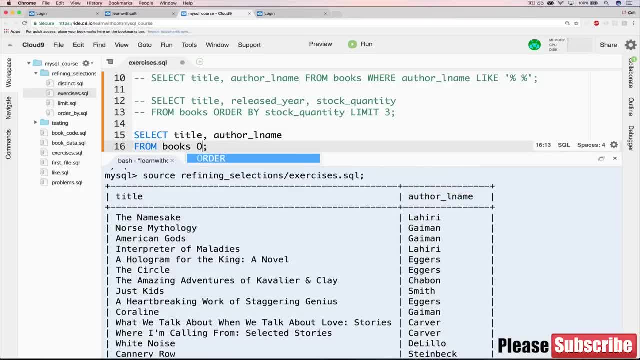 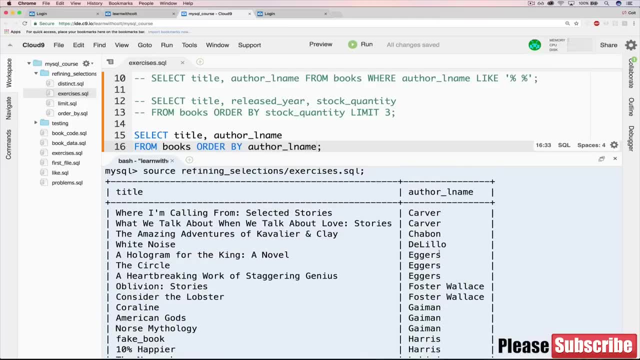 So now let's sort by the author last name. So that's just a simple order by author L name, And that gives us the alphabetical order we're looking for. So we don't need to use descending. That's all right. But then, if you look over here, if we take Carver's, 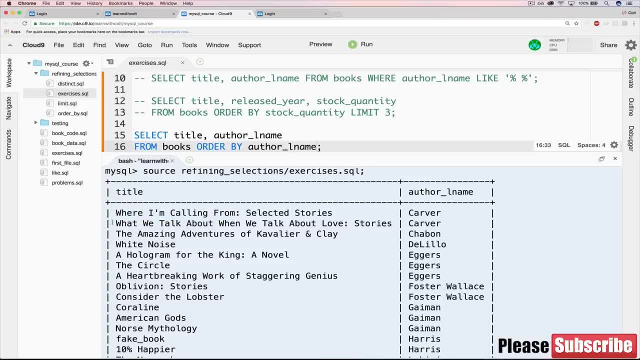 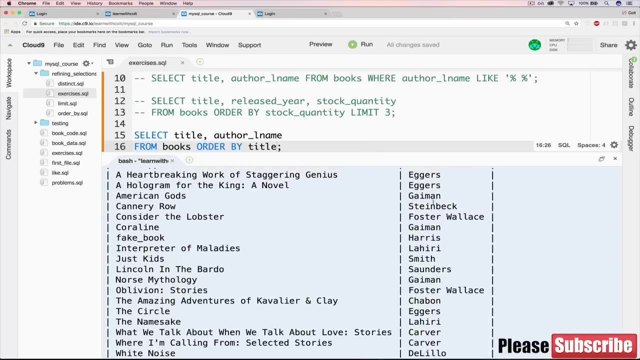 books. notice that where I'm calling from comes before what we talked about when we talked about love, even though WHA comes before WHE. So we want to now sort by title there, And the way we do that is not by just changing that to be title, because then it purifies the title. So we want to now sort 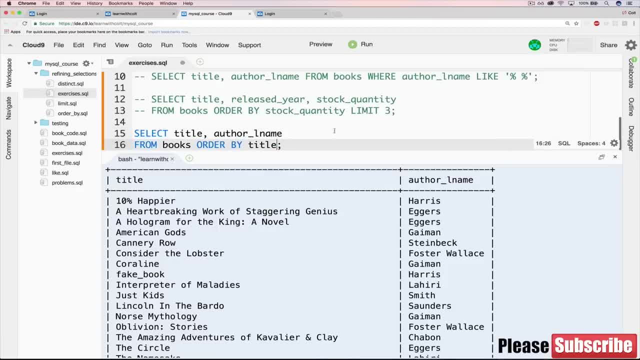 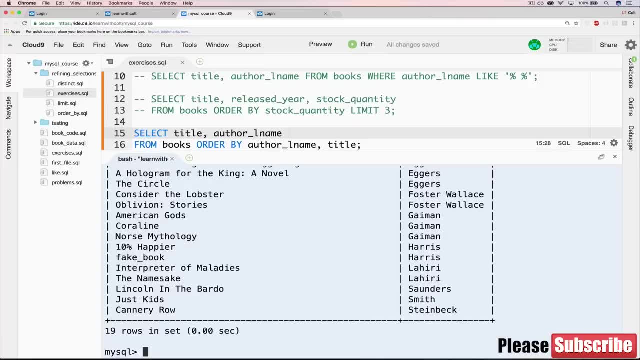 by title and ignores author L name. Rather, we want to do this: author L name, comma title. And there we go. Now you could also replace this whole thing with two comma one, which I really don't like, just because it's not very semantic. It's not meaningful to look at this. 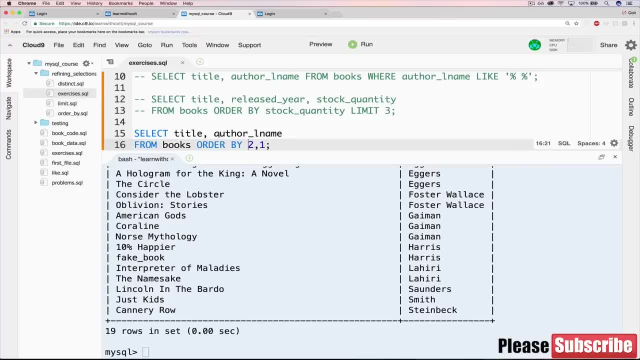 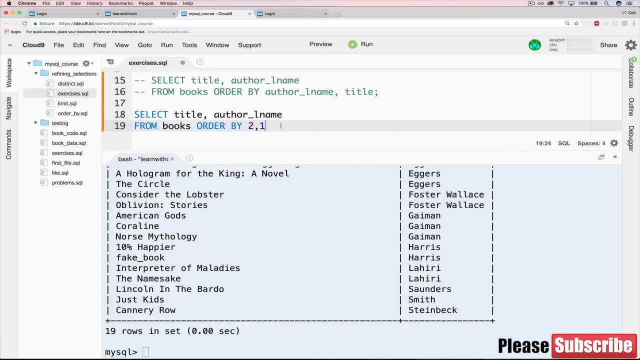 But it is shorter, And again that two is referring to author L name and one is referring to title. It's just the order that we're selecting them in, So I'm going to change it back, But I will also duplicate that below and change it to two comma one And comment that out as well, just so. 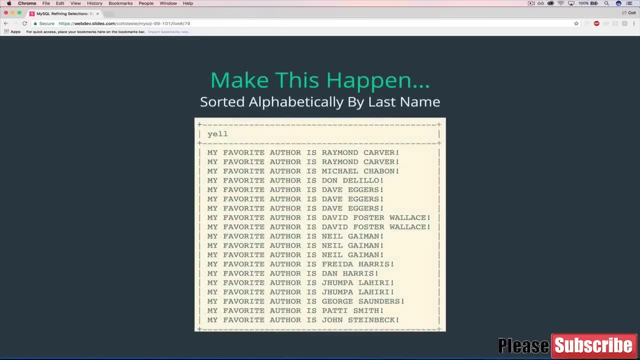 we have both solutions, Which brings us to the last problem. Hopefully it's the last. Okay, it is. make this happen. So we want to yell. my favorite author is. and then the uppercase first name of an author and then a space in the uppercase last name of an author. 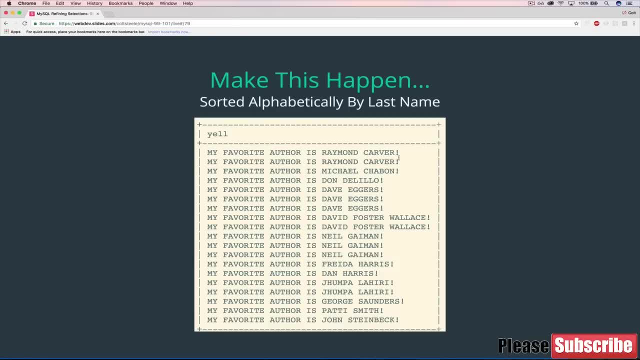 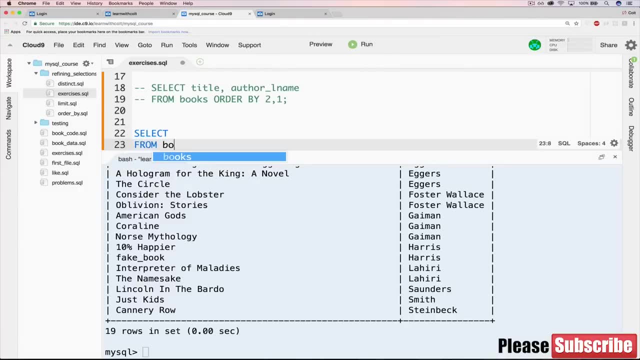 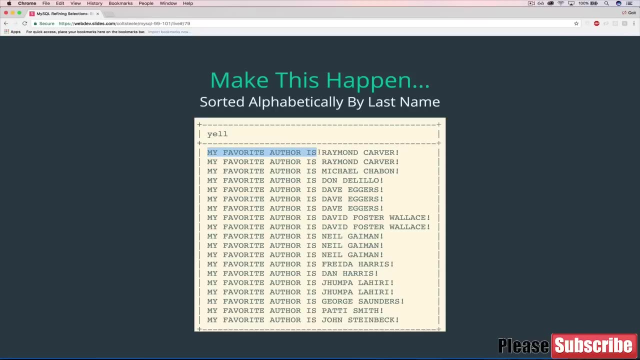 And then exclamation point. Yeah, it's kind of a lot. Okay, so let's start with selecting, And we know already that well, we can start with select from books. Sure, What we're going to want to do is concatenate- my favorite author is- and then an uppercase. 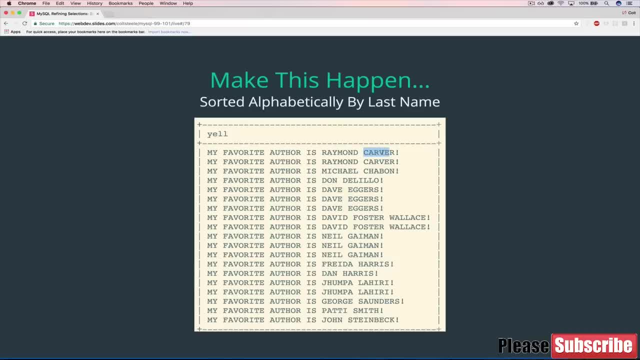 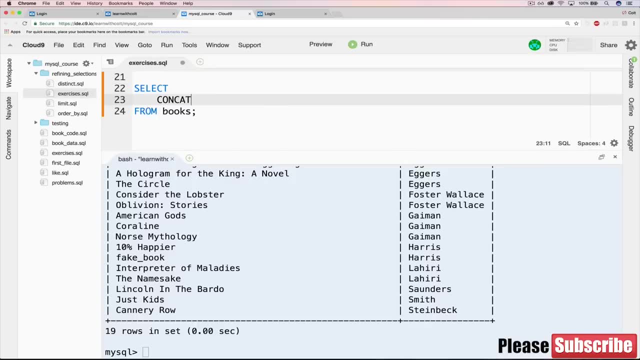 version of Raymond and a space and then uppercase version of the last name. So, and exclamation point, it's a lot of concatenation, So we're going to have a concat And I'll just do this. Oh, let's do this way, Just like that. What are we concatenating? Well, 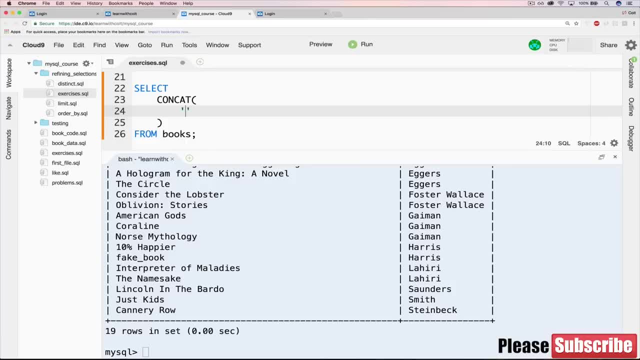 let's start without the uppercase or without. So let's just start with my favorite: author is, and we'll add a space comma, and then we want author F name, And then we want another space, this space here, so they don't just run together. 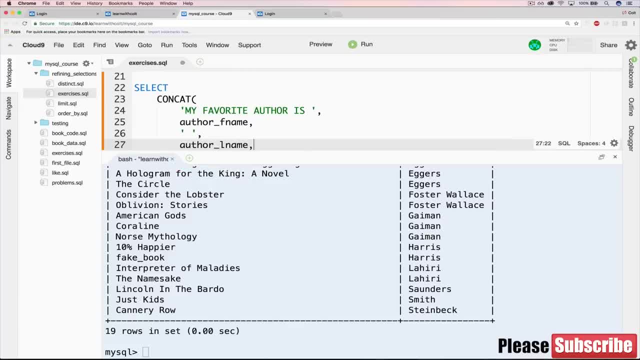 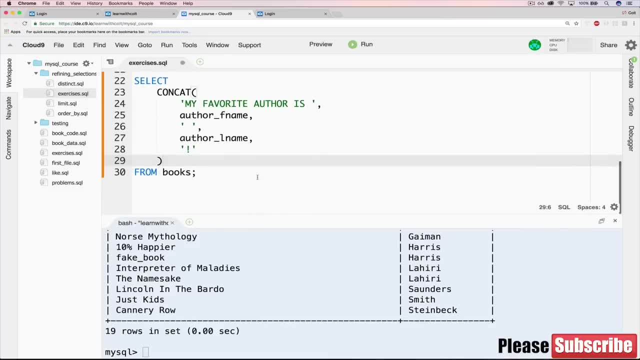 comma. author L name. Finally, an exclamation point. It's a lot So let me drag this down a bit so we can see the whole query. Select the concatenation of my favorite author is: space, the first name of an author. space, the last name of an author- exclamation point. Let's save it and 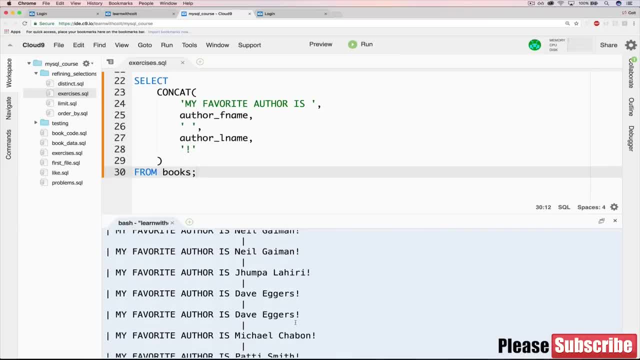 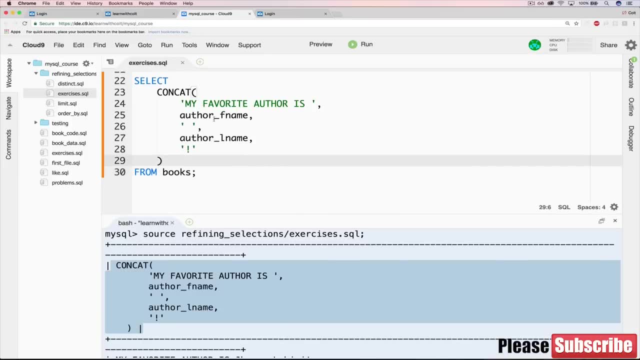 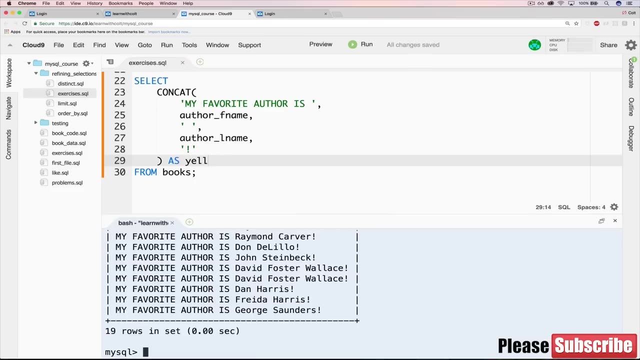 run it. It's pretty long. Oh, and this is partially messed up because you can see up here the column heading: here is this entire thing, So let's add the as yell. Now, if I run it, there we go. 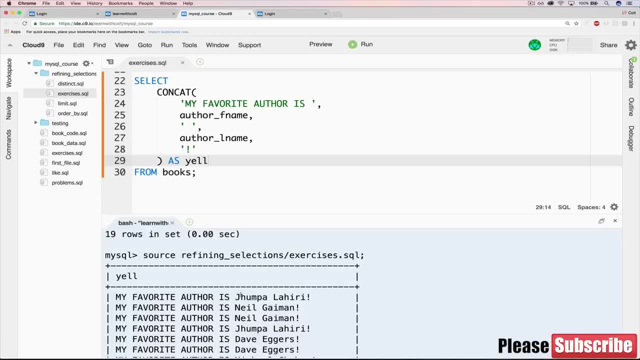 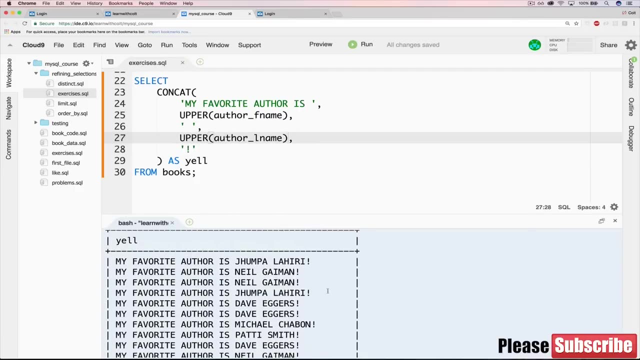 Okay, So we're close. The next thing we need to do is capitalize author F name and author last name, which is easy, Just an upper like that. Save, rerun it. Okay, It's all uppercase now. 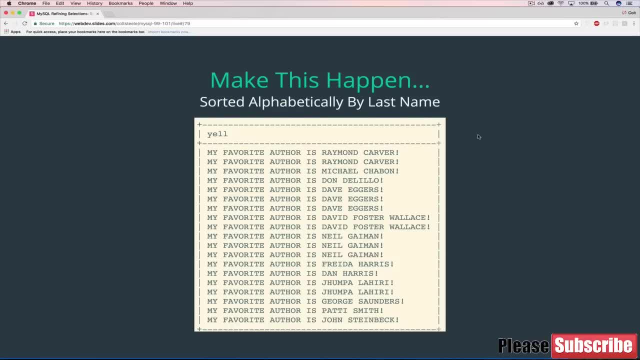 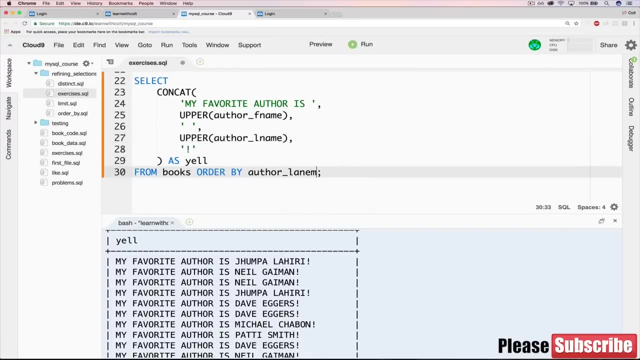 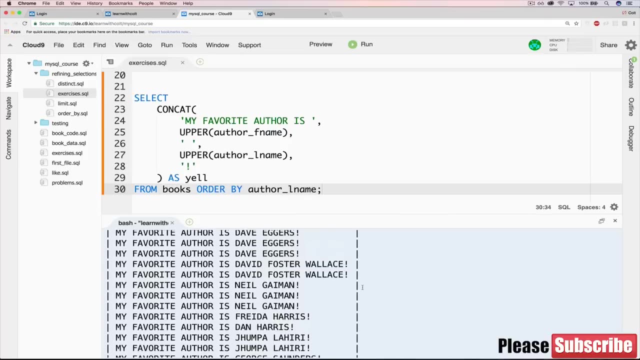 We have one last thing, Which is sorting alphabetically by the last name. So from books, order by author, L name Long query here. Let's try it. It looks like it worked. We got Raymond Carver all the way down to my favorite author is John Steinbeck, And that's about as loud as I'll yell. 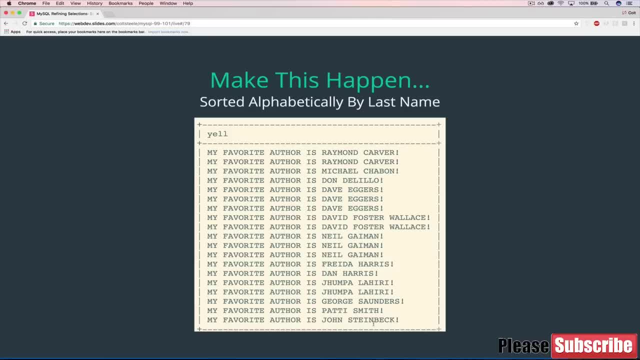 in here. Don't want to wake my neighbors, All right, So congratulations. Hopefully you made it through this relatively unharmed. A lot of exercises, a lot of ordering by and limiting, But the reality is you will use those a lot. It is very useful to be able to determine. you know the, the, I mean highest page count. 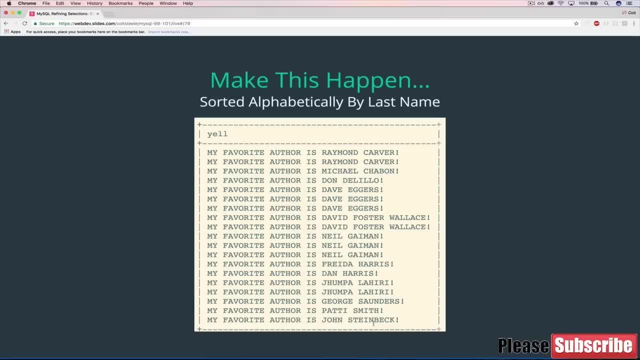 maybe not, but the best selling book. once we get to to sales and users and stuff for the most active users or, like I keep coming back to the highest commented post, or the most trafficked, the most clicked on ad, all those sorts of bits of data are really useful And you'll use order by 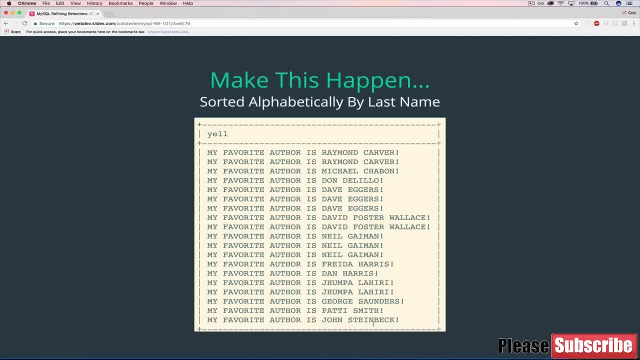 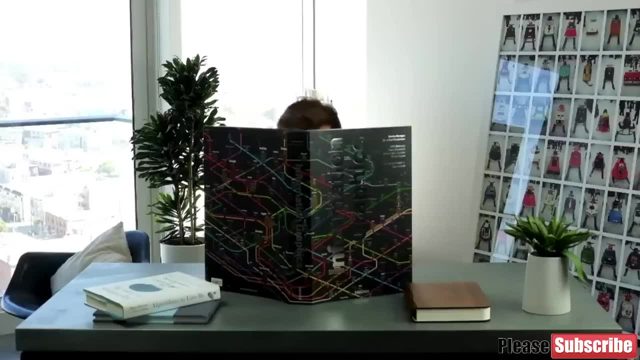 and limit all the time, as well as other tools that we saw, distinct and like. they're all very useful, All right, Well, I recommend you take a quick little break and then we'll move on. Hey, Hey, welcome to the next section. So this section, as you can probably gather, 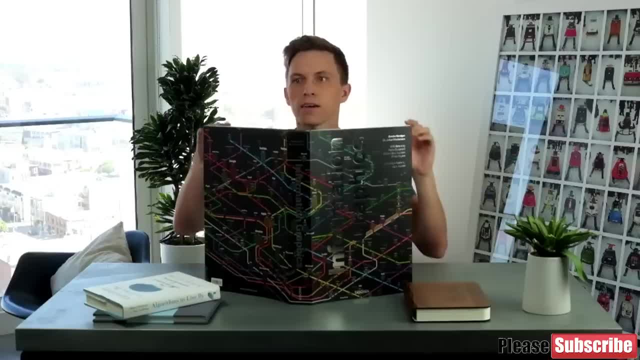 we're still working with our books data. I hope you're not tired of it yet. If you are, we're almost done. But it's important that we keep working with one data set, for a little bit at least, so that you can get familiar with it, And the reason that that matters is that 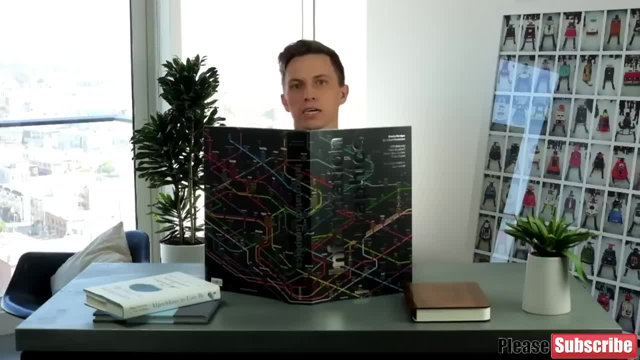 is that, as we do some of the more advanced things, we want you to be able to check your work. So in this section we're going to learn a lot about different ways of performing analysis on data. So things like finding averages or summing a bunch of data together. 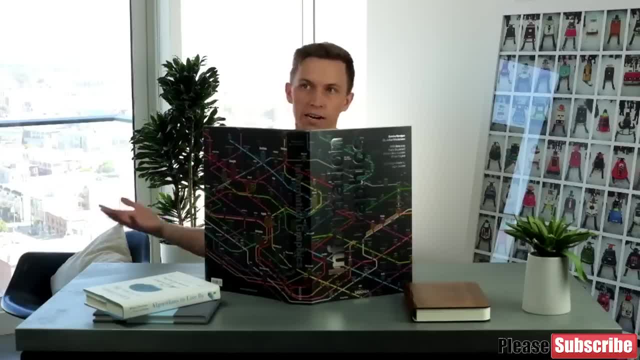 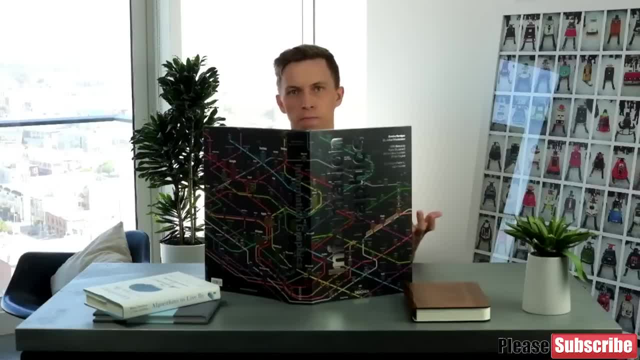 let's say 67.5.. And how could you know if that's right or wrong? But if we're working with books and we have 20 of them and you're familiar with the page counts and the authors, you'll know: okay, this author has three books. that seems right versus okay, that author only has two books. Why. 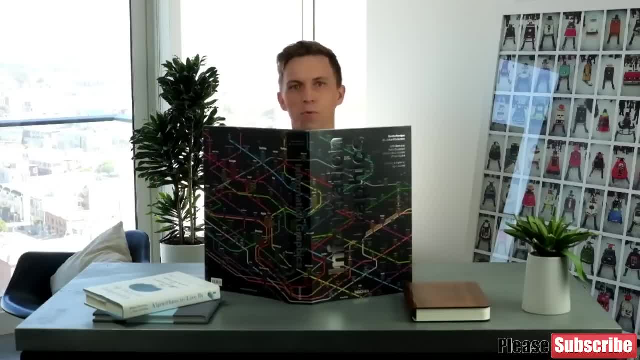 are we saying that? you know we have three or something like that Terrible example. but the same idea is true: We know our data. at this point, We're going to at the end of this course and, along the way you know, we're going to keep upgrading our data to more complex. 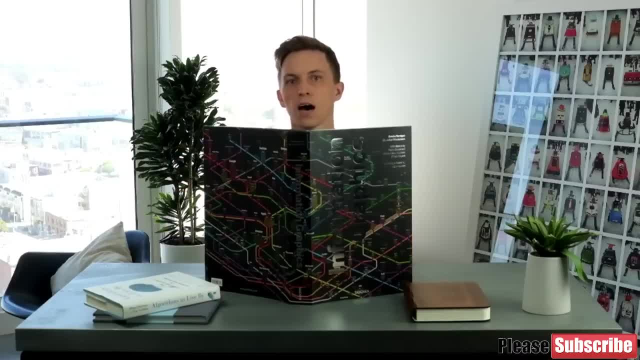 structures, more tables, more rows, complex stuff. But at the very end, kind of the capstone case study, we'll be working with Instagram-esque data- fake data for Instagram- And we'll have thousands and thousands of rows And you won't actually know if you're doing things right or wrong, based off 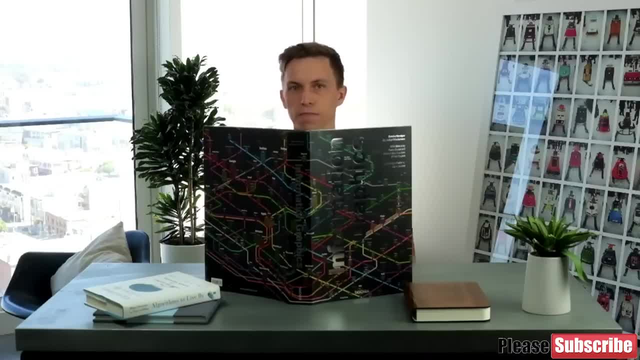 the number you're getting, unless you've manually checked your work by, you know, doing a thousand additions or something. So all that's to say, stick with the books if you can. And in this section we're focusing a lot on these new aggregate functions. So those are things like finding 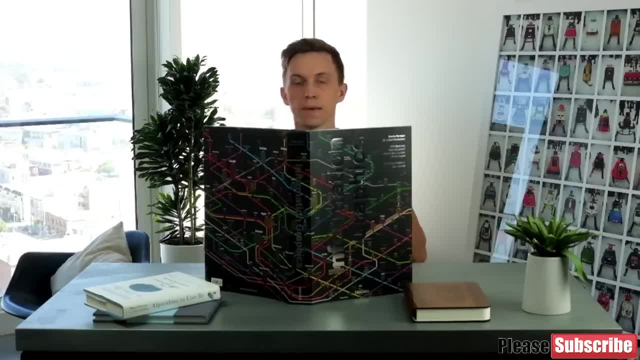 averages, counting, summing things together, based off of grouping data. So it's a bit hard to explain in a headshot without showing you code, So I'll let the code do that in just a few videos from now. But the rough idea is that we take our data and there's all sorts of insights we can gain. So 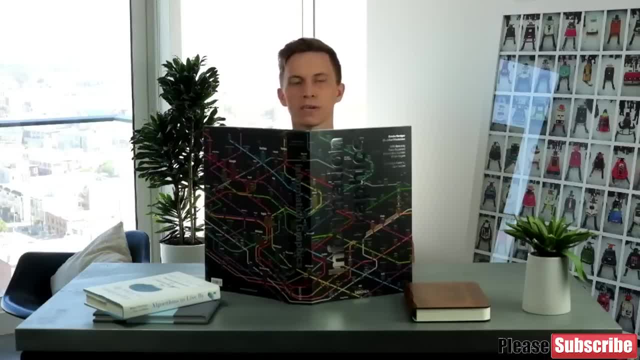 rather than just working with an individual row or a group of rows, we can combine things into like ego rows. I can combine all of our authors and group books based off of who wrote them, or group books based off of what year they're written in, and then perform operations on those groups. So it 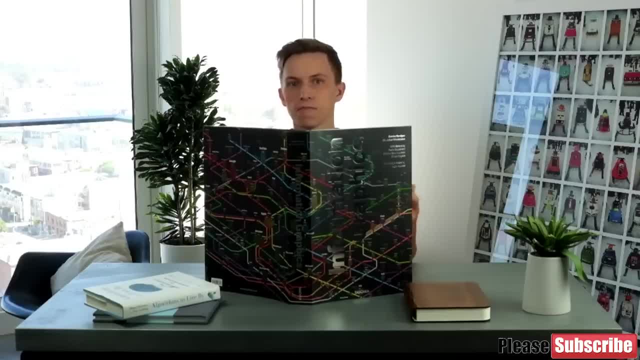 allows me to do things like find the average sales that we've had per year. or we could do things like find the average page number for books per genre, And then we could expand that obviously to more complex stuff if you're working with advertising data or, let's say, our Instagram data. 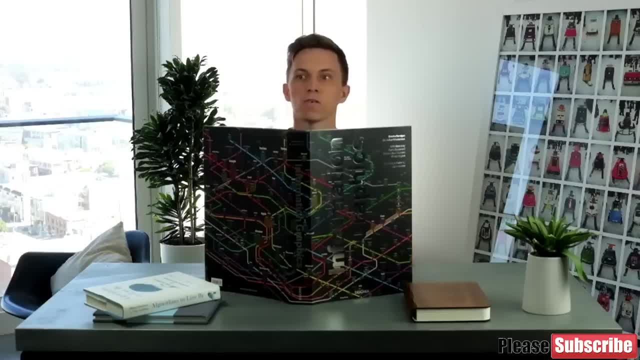 We'll be able to, at the end of the course, do things like find out which one of our users is a power user- influencers, what they're called, I guess, meaning that they have the most comments, the most likes on each one of their posts on average. So who in our database is getting? 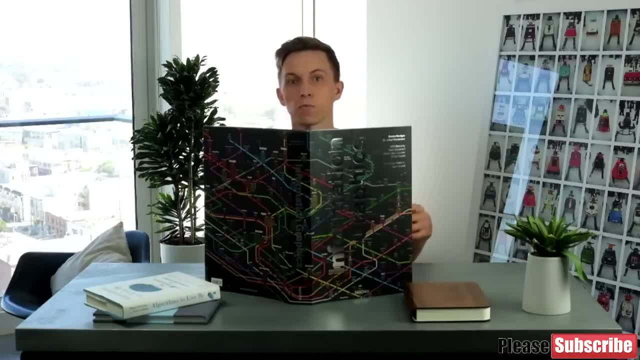 on average, the most likes and comments. Or we could do things like which hashtag generates the most traction, And to do that we would need to analyze all of our hashtags and then take all of our photos that have those hashtags, group them together. 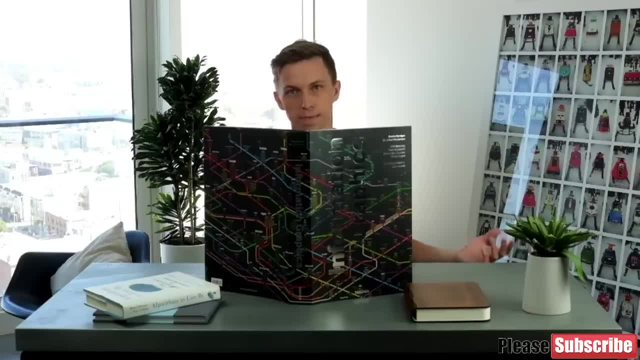 figure out which one of those hashtags generates the most likes. So there's a lot of stuff that we can do with these aggregate functions. They form the backbone of a lot of the questions and analysis that we'll do throughout the course. All right, I'm rambling. now I'm going to go away, Hopefully. 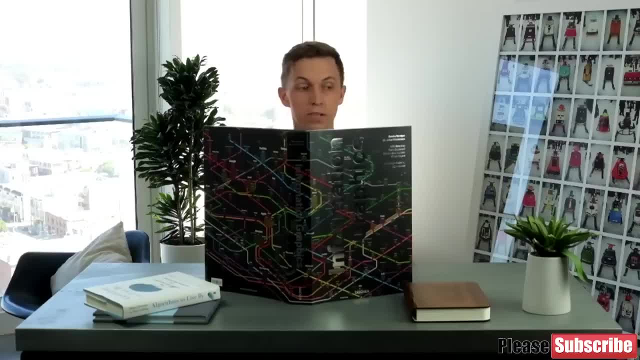 you enjoy this section. It's important- I say that a lot, but it really is- And of course we'll have a bunch of exercises throughout the course or throughout the section and especially at the end, And I'm trying to keep those interesting. Look forward to those, If you. 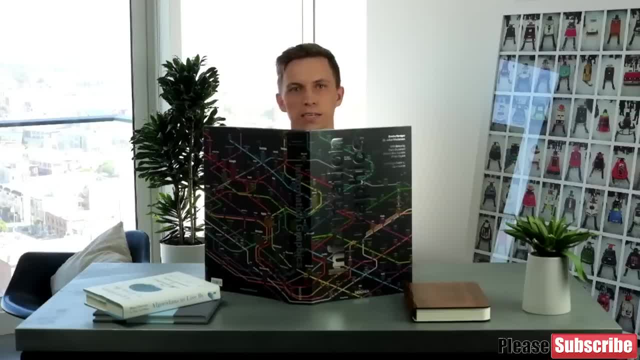 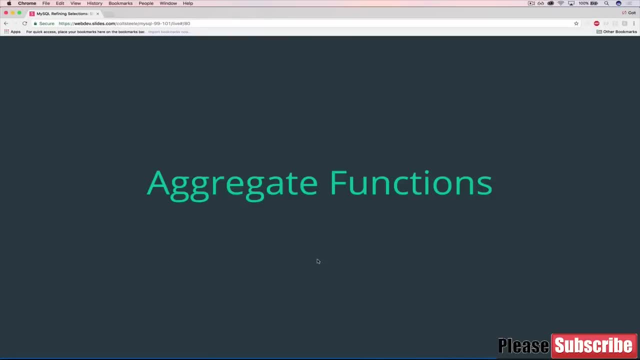 just remember it's a database course. I'm trying my best It's. you know it's databases. All right, I'm done. Alrighty, then Welcome back everyone In this section. we're kind of continuing with the trend of focusing on selecting our data on reading it. 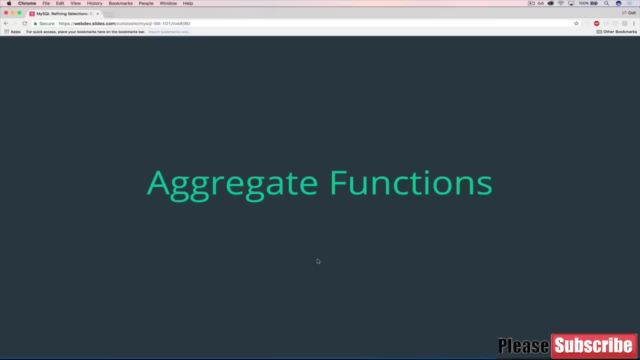 if we're going back to CRUD. In the last section we saw things like sorting with order by using limit and so on. In this section we're going to focus on what are called aggregate functions, And basically these are built-in functions in MySQL that will allow us to aggregate or combine data. 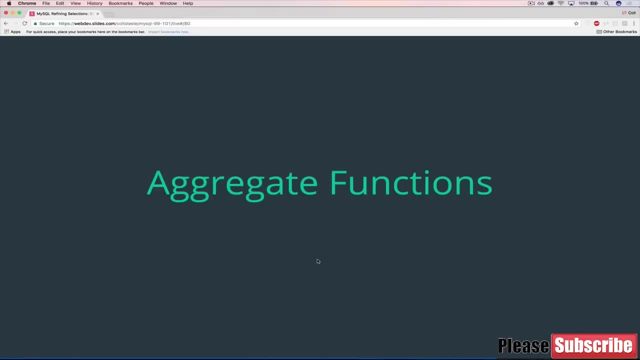 to get meaning out of it. So by the end we'll be able to do things like find the average page length of all of our books or find the average page length for each author. So you know, let's say we'd be able to tell that someone like Carver, who writes short stories, 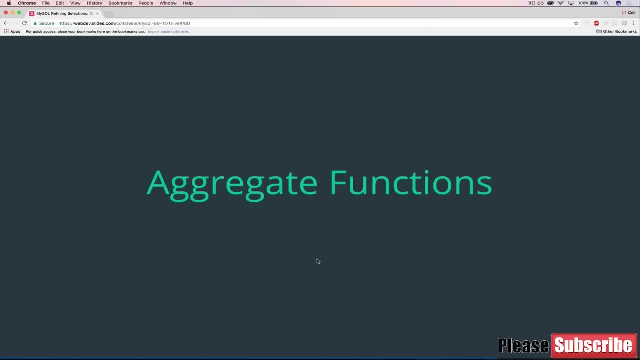 maybe has shorter books compared to David Foster Wallace, And that's just average, but we'll see. We'll see how to do other things like count, sum, min max and a bunch of others, And they're known as aggregate functions because they work on aggregated data. So yeah, let's get started. 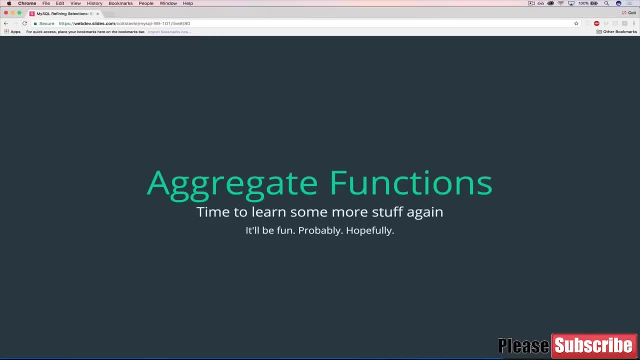 It's time to learn some more stuff, And it will definitely 100% be the most fun thing that you've ever done. Let's get going. The first thing we're going to take a look at, the first one of these aggregate functions is called count, And it does pretty much what you would expect, at least in the 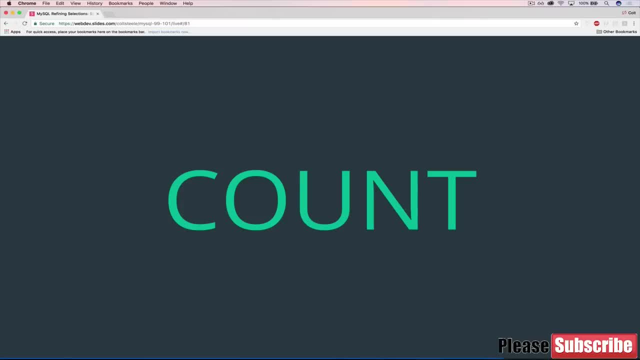 way that we're going to show it to you now. We're going to revisit count in the next video, once we introduce what's called group by, But for now we're just focusing on count on its own, And what it will do is count whatever you tell it to count. So here's an example. 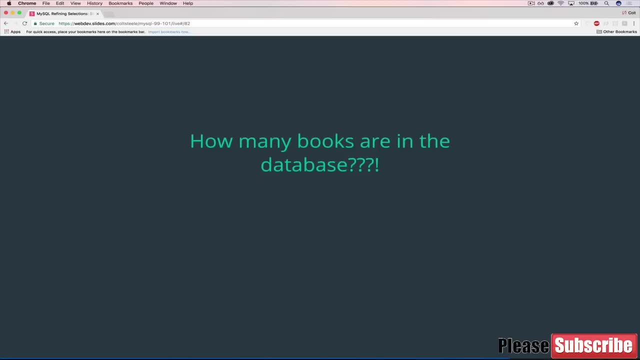 How many books are in our database. If we wanted to do that right now, you could do a select star from books and manually count which technically would I mean that would work. But if we have, you know, Amazon's database that has millions of books, that would be. 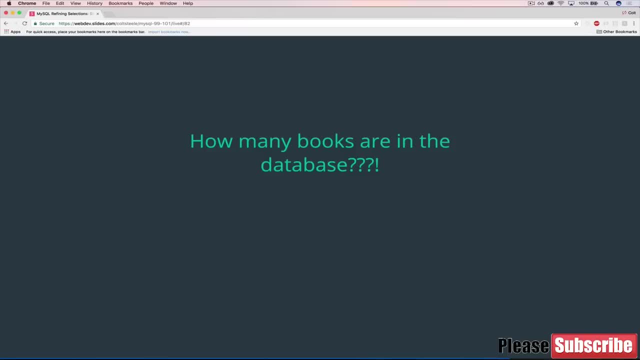 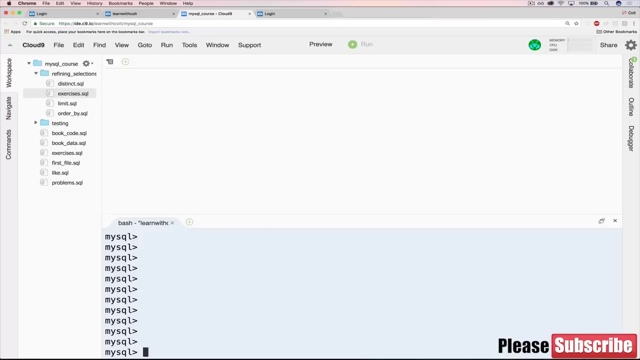 a lot of work. That would take at least a couple thousand mechanical turks to do, so. that's not ideal. instead, we can use count, and it just looks like this select count star from books. so let's try it and then we'll discuss it a bit more. so here i am. i'm using 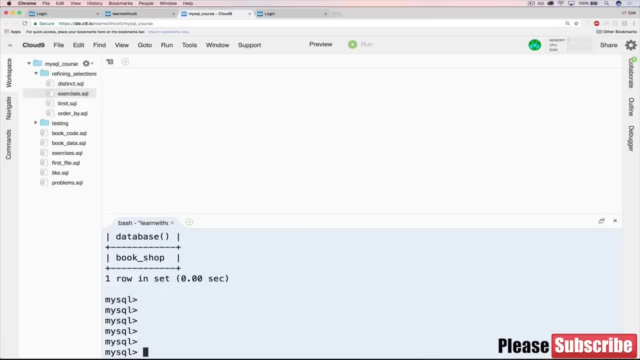 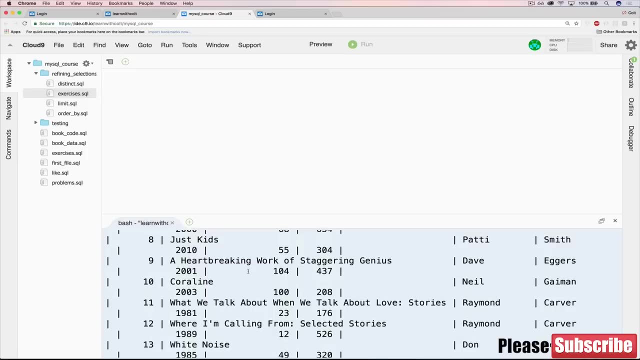 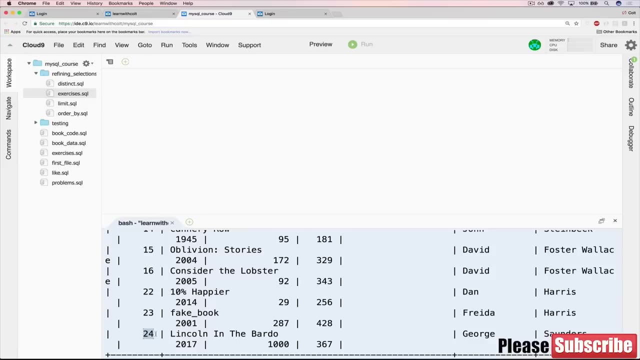 the same database, just double checking bookshop, so we can do a select star from books and, like i said, we could go through and count, um, and you can't just rely on the ids, of course, because we could have deleted some. so just that the highest number of the id is: 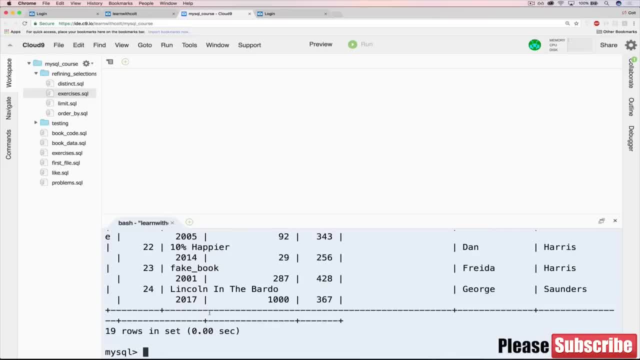 not a reliable way of knowing how many books are in there, because when you delete something those ids don't change, they don't shift down. so instead we do a select count and we'll put star here, which basically will count every row, the entire row. so select count. 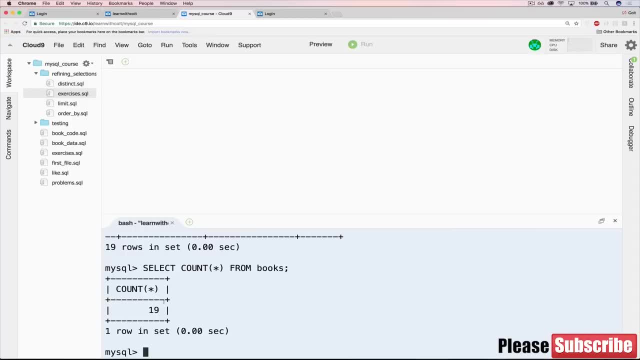 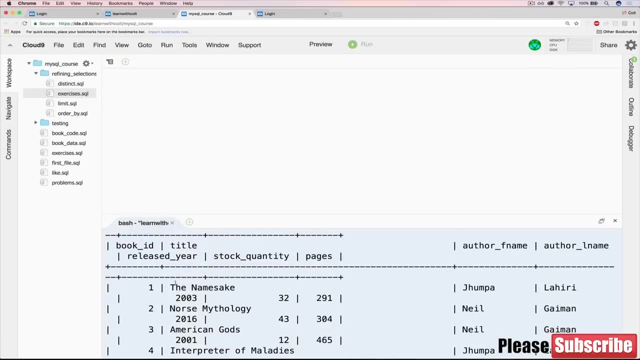 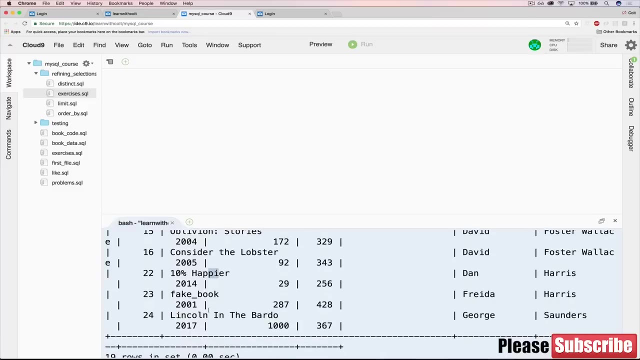 star from books and we get 19.. so that tells us there are 19 books, and we could verify that, you know. let me just uh speed this up as i count one, two, three, four, five, six, seven, eight, nine, ten, eleven, twelve, thirteen, fourteen, fifteen, sixteen, seventeen, eighteen, nineteen. all right, so there were 19 books. 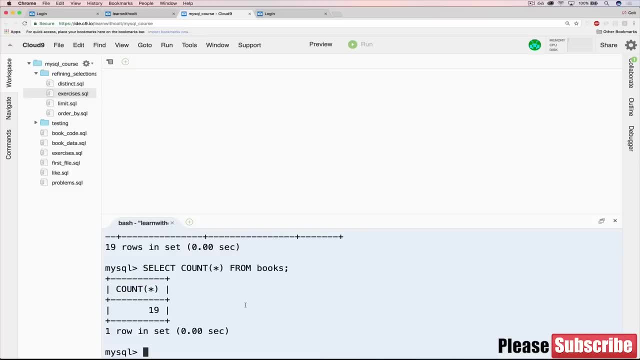 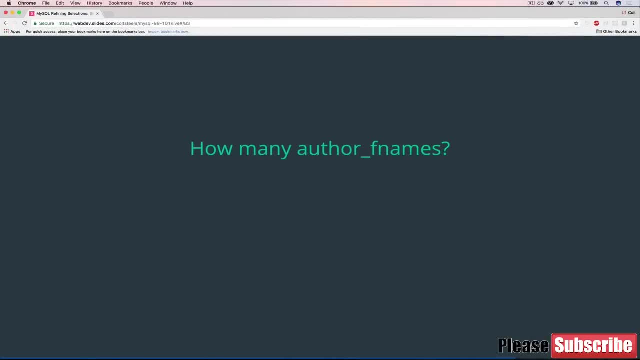 so we can trust this count. it's right, um, and that's one way of using counters to check how many things are in table in general. a more specific way of using it, we're going to be to do something like this: how many author first names are in our database? and it's not. 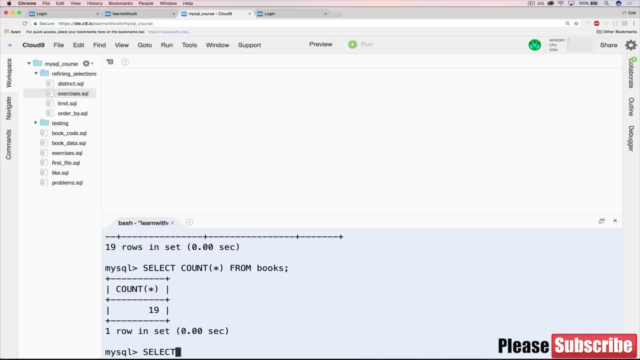 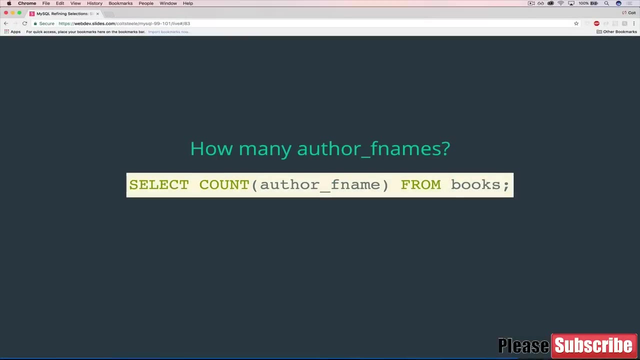 19. we know that now because if we do a select author f name from books, you know we have some authors who are in here multiple times. neil gaiman is in there twice, so it's going to count them twice. it's just going to count everything here. so if we did this select count author f name from 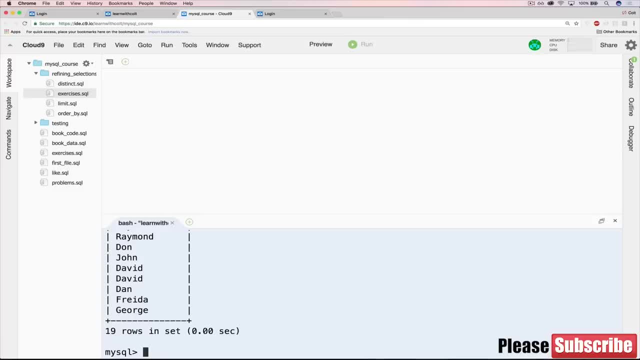 books. is it really going to be correct? and the answer is no, as i just said. but let's just try it. select the count of author l name from books, or we're doing actually f name, aren't we? and it tells us there are 19 author f names, and that's technically true. there are 19 f names in. 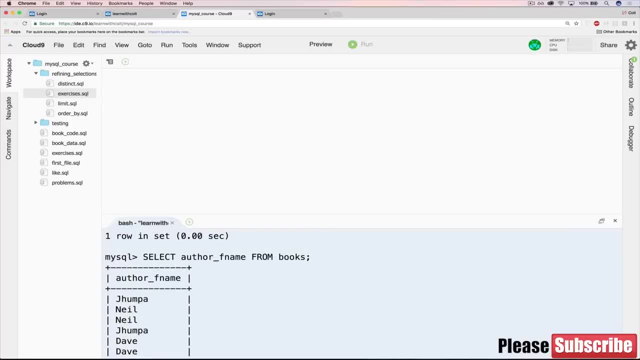 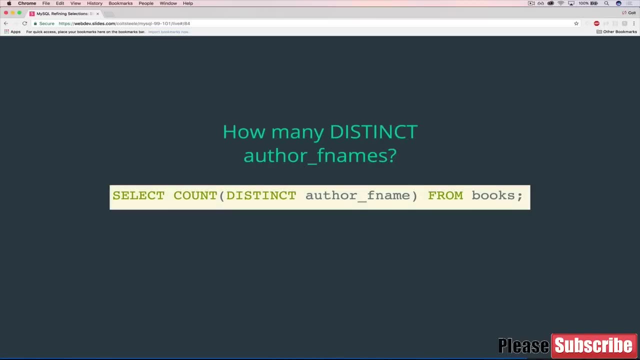 here. i want to know how many unique first names are in there. unfortunately, there's a way of doing that and it relies on distinct, which we've already seen. so we just put distinct inside of that count. so select count, distinct author. f name from books. let's try it: select count, distinct author. 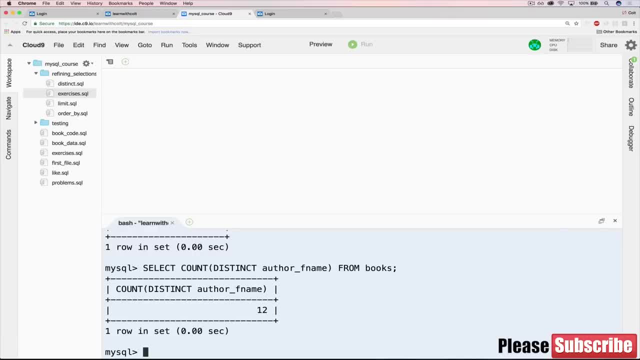 f name from books. and now it tells us 12, and i won't make you sit through me counting it, but there are indeed 12 first names that we have in our database. so instead of 19, it's now decided: okay, there's. there's only one here, and there's one here, and there's one here. 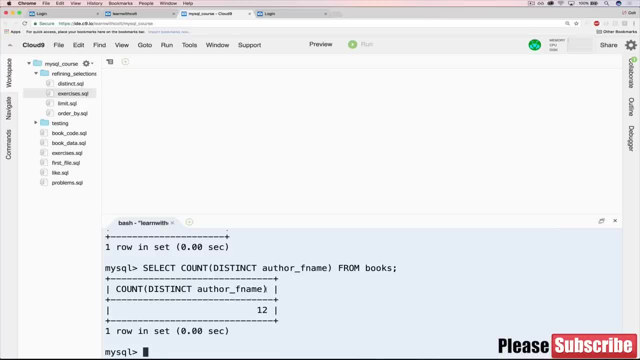 So that's the basics of using count, along with using count with distinct. Now I do want to show you a bit of an edge case here. Let's say I wanted to know how many unique authors are in my database. So that means first name and last name. So if we do our select count and let's just do author last, 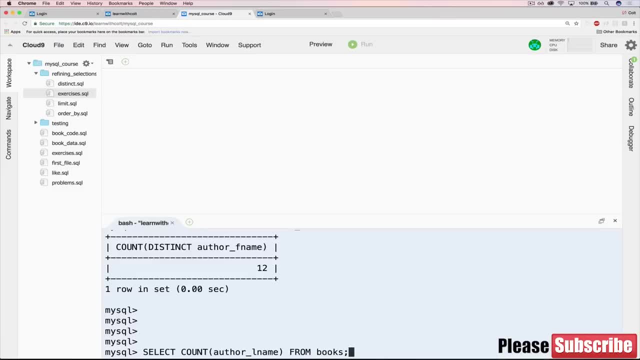 name first. from books we get 19.. As you would expect, there's 19 rows. every row has a last name, But we know that there are some duplicated last names and if we just look at those, just do this very quickly- it's the same problem that we had with first name. right, We had Foster. 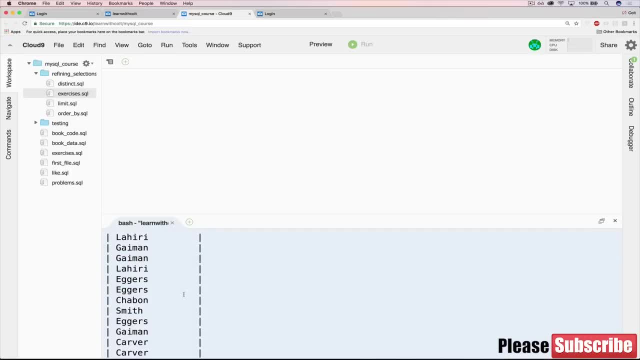 Wallace, we have Eggers and we have Gaiman. So if we use that distinct select count, distinct last names, maybe you can see where I'm going here. If I hit enter, it tells us there's 11 distinct author last names, which is true. There are 11 distinct last names. 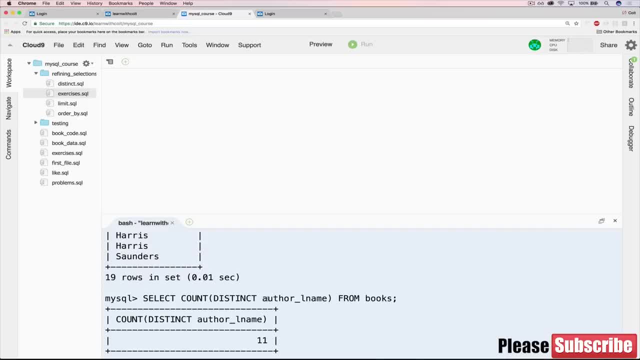 but that doesn't mean there are 11 distinct authors, Because if we go and do a select author fname, comma, author lname- so if we look at both first name and last name from books, remember that we have Dan Harris and Freda Harris. So when we're selecting distinct last names, it treats this. 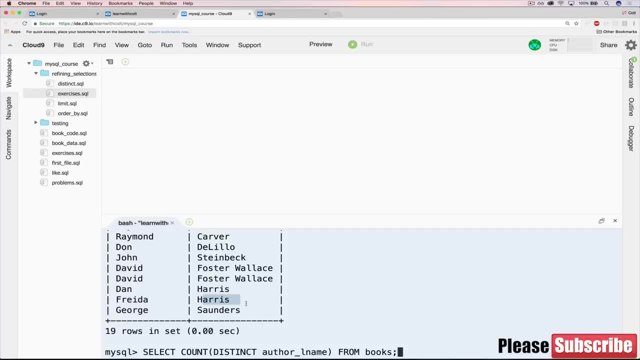 as the same, because Harris is the same as Harris. So if we wanted to know how many distinct authors were in there, what we could do is do author lname comma, author fname, And now it's only going to return distinct rows where first name and last name or last name and first name are distinct. 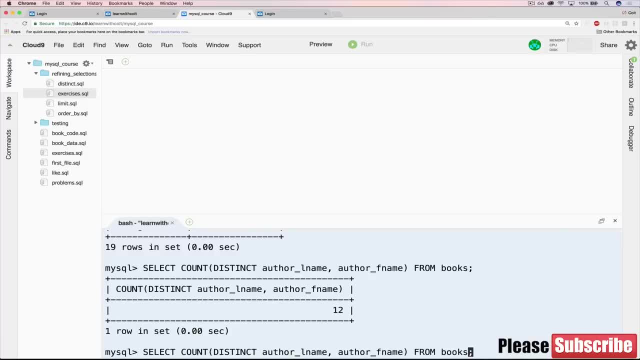 That gives us 12. Which in our case, is the same as just doing this right here. As we just saw, if we only do author fname, we can see that we have Dan Harris and Freda Harris, So we can use that as an. 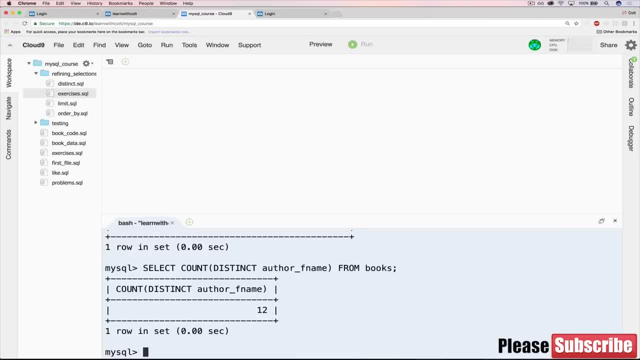 F name, But that's because we don't have any duplicated names or any duplicated first names in there. We have David Foster Wallace, but we don't have, I don't know, David Johnson or something, So this would be problematic if we had multiple Davids. So then we could use this. 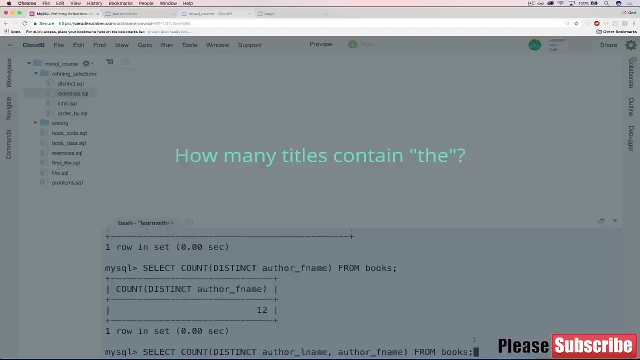 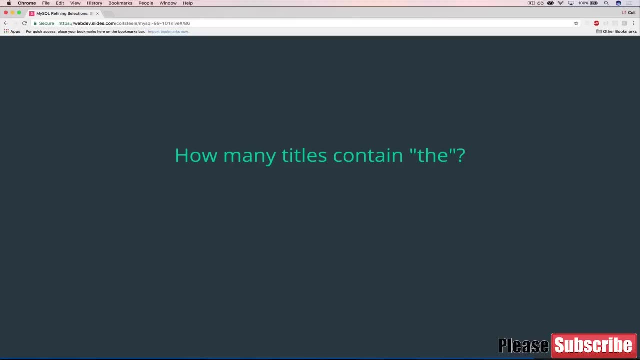 where we're doing distinct author L name and author F name together, And the last thing we'll do is this question here: How many titles contain the, the string, the T-H-E? So if you'd like to make this a little bit of a mini exercise, go ahead and try it. How many titles contain the? 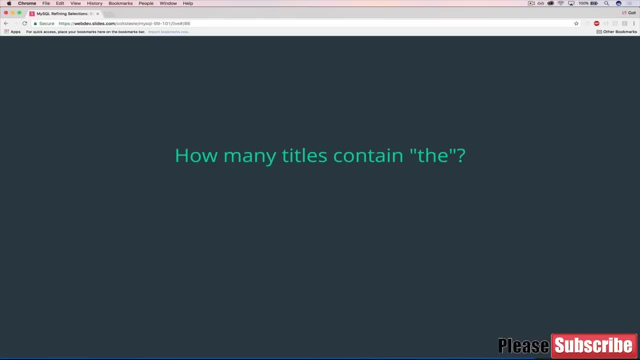 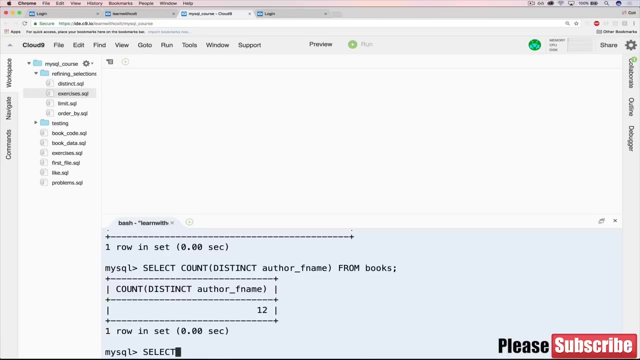 in the title, or how many books title contains the, And the answer is that we need to use like alongside with count. So let's do it now. We're going to do a select and let's just start by selecting the books, the title from books where title like, and then this is where we need those. 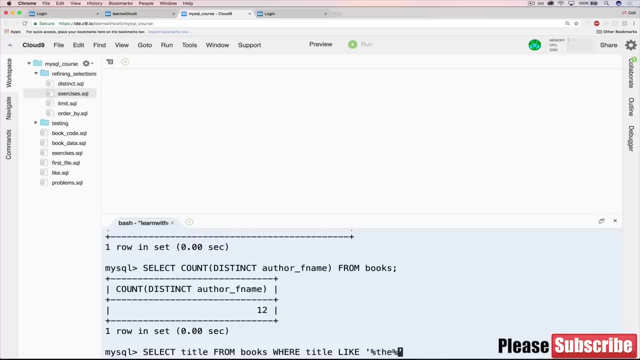 wild cards T-H-E. we need a wild card on either side. All right, and here we go. We've got the namesake: the king, the circle, the amazing, the lobster, the bardo Great book, by the way. So there are. 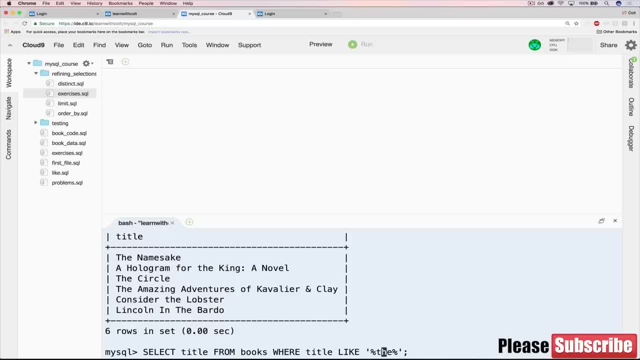 six of them here, right, Yes, So if we wanted to do that with our code dynamically, not by counting ourselves, we would just replace that with a count Select count from books where title is like the and it tells us there are six. All right, So I just wanted to show you you can combine it just. 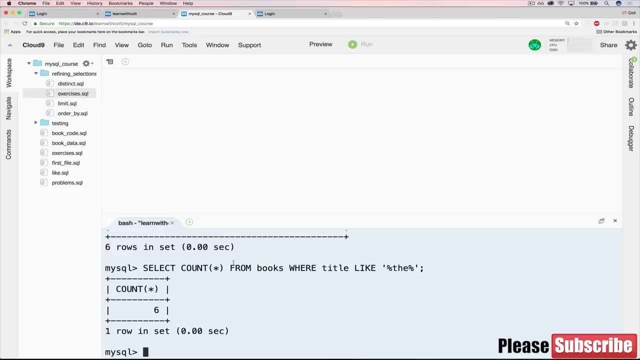 like you can with any other of the things that we've seen. So you know, substring or concat or upper, they work the same way. In this case we're just selecting count, All right. So that's count. Next up. we're going to go a little bit off the rails and talk about something called group by. 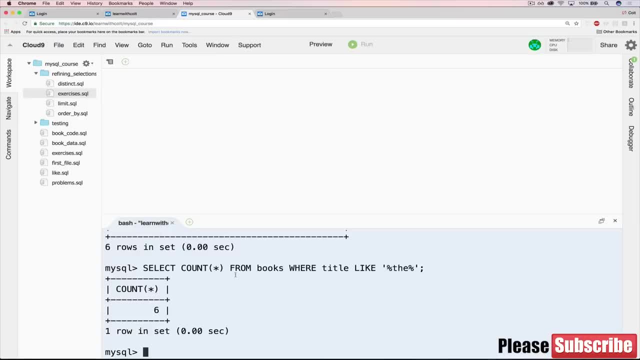 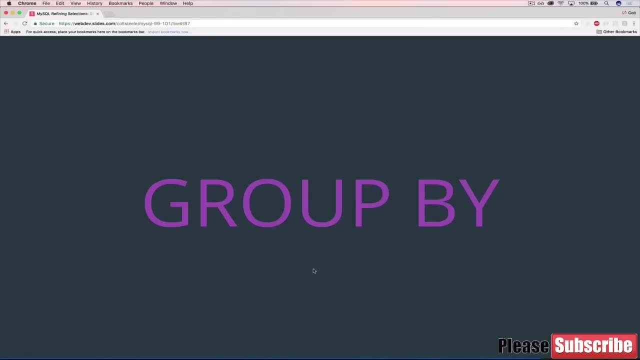 brace yourself. It's- uh, it's refreshing, Let's put it that way. Okay, So next up, we're talking about something called group by, and group by is is going to be essential to everything we do in the rest of this section. 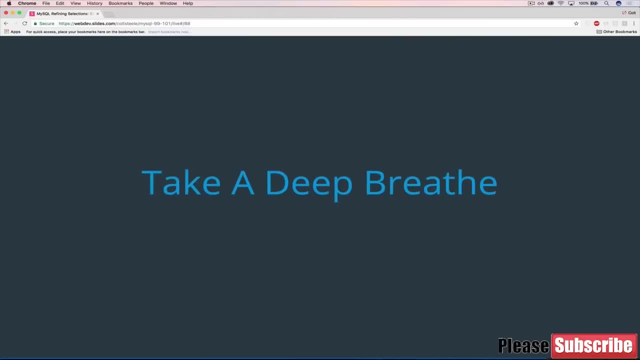 Um, and I'll warn you right now- take a deep breath- that it's a little bit weird. It's different than the things that we've seen so far And, in fact, for me personally, it's a challenging one to teach because, like like I just said, it is different. Um, it's not just a single little function that 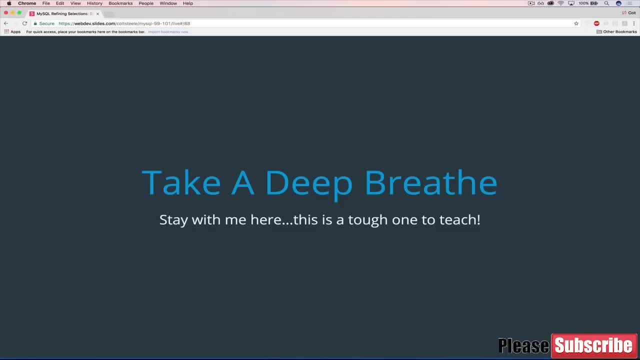 we can throw in there like concat or upper, where we get a nice immediate impact, where we can see: okay, that was uppercase or that was concatenated, Uh, or that's a count. rather, we have to use it alongside some other functions, So it's going to. 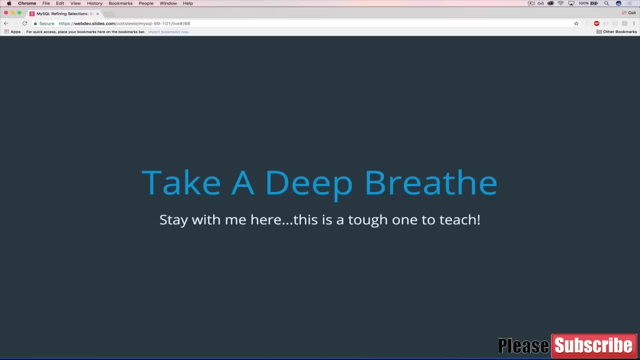 take a little bit to explain. So hang in there and just know that we're going to get there. There is a payoff and it is very useful. It's kind of at the core of aggregating our data. It's how we can do things eventually, like average or some, or find the minimum or the maximum and so on. So here we. 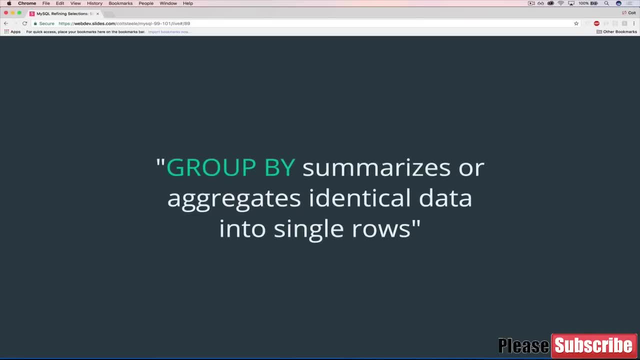 go. This is a little blurb that I wrote uh about group by group, by Summarizes or aggregates identical data into single rows, So it's actually pretty self-explanatory. The name group by we can say things like: take all of our books and group them by the year they were. 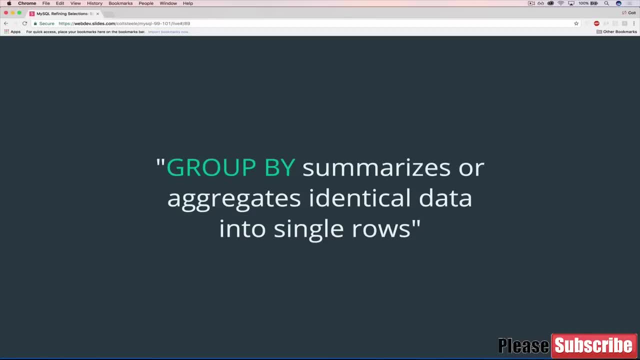 released, or group them by the author last name, or take all of our teas, or actually, let's say, take all of the movies in our database and group them by genre, And that on its own is not that useful. but then we can say things like: group them by genre and tell me how many each genre has. 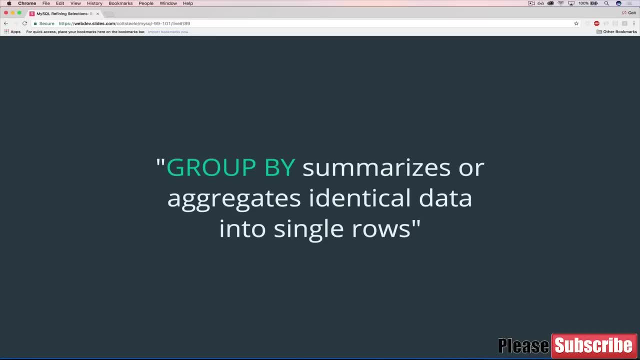 Or group our teas by variety, like green tea, white tea, black tea and so on. Group our teas by variety and find the average sales price for each one for each variety, that is, or add together all the sales for each variety and figure out which tea type is selling best. So we'll get there in. 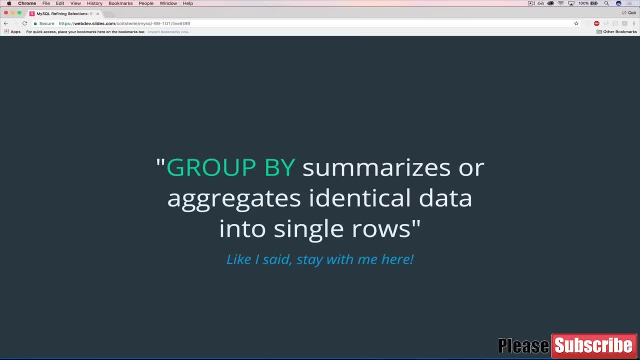 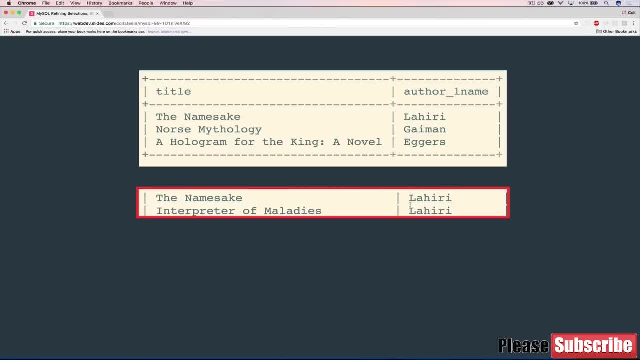 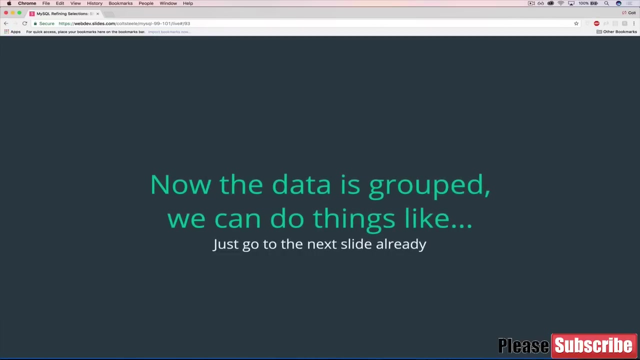 say we're working with a very small variety of tea. Let's say we're working with a very small variety of tea. Let's important because the data is now grouped and we can do things like this: count how many books each author has written. so our query would look: 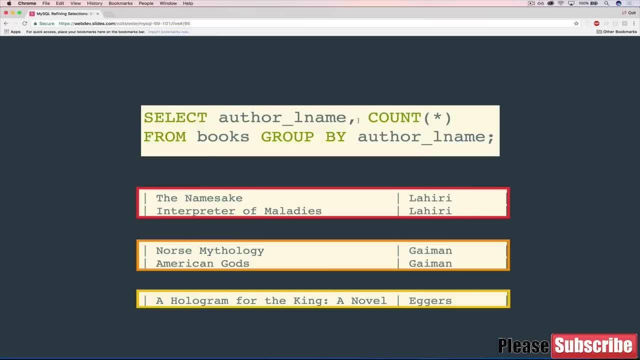 something like this: select author last name comma. we don't have to have this here either, but it's like the author last name comma, count star from books grouped by author last name. so it's going to group them like we've already seen, and then when we do a count star, it's not going to count every row in our 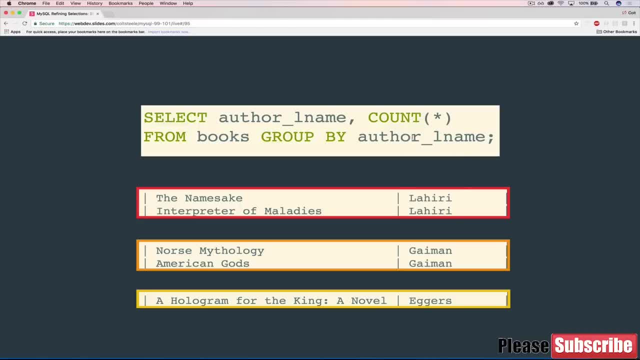 entire table. what it's counting is, for each of these mega rows, how many sub rows are in there. so, basically, how many things are under Lahiri- and in this case there's two- how many things, how many books are grouped under Gaiman two and how many are under Eggers one? so then, what we get spit out when we're actually 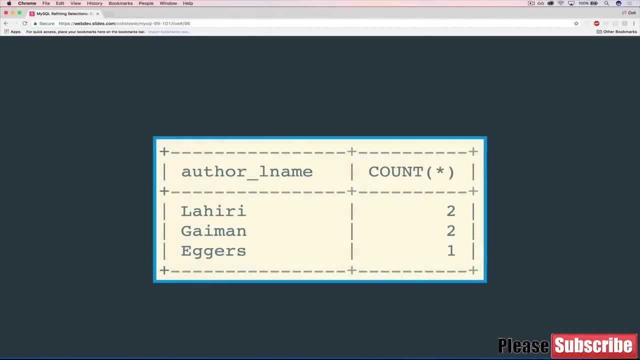 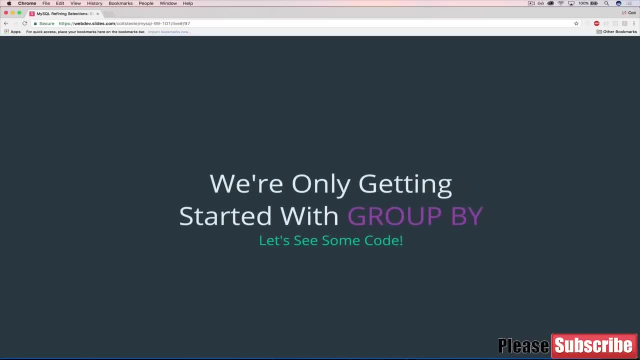 selecting the author: last name and the count is this: Lahiri two, Gaiman two, Eggers one. so we're only getting started here with group by. I'm gonna now dive into cloud nine and do some more, but just know that we will be using group by to do things. 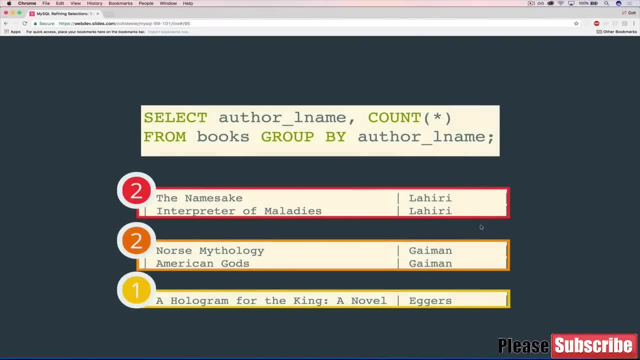 like average. so once we have, let's say, grouped by authors, we could average the page count, like I said, or the average year that they wrote a book, or we could find the first year they wrote a book using min, which we'll see in just a moment, where we can some the total page count, for instance, for every. 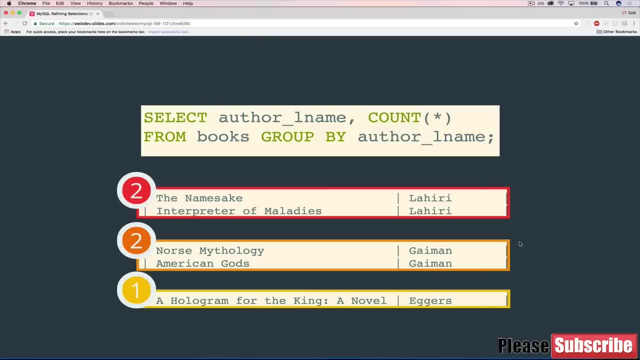 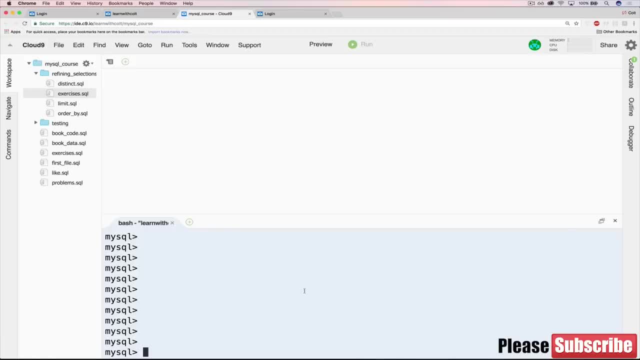 author. so group by is very important and versatile. for now we're only using it in conjunction with count. now let's dive into cloud nine and do just that. let's start with something simple like select title comma, author, lname, but you actually first name and author, last name from books, so no counts overflow in the third types. so group by and second times our By name for theаєu and Command. 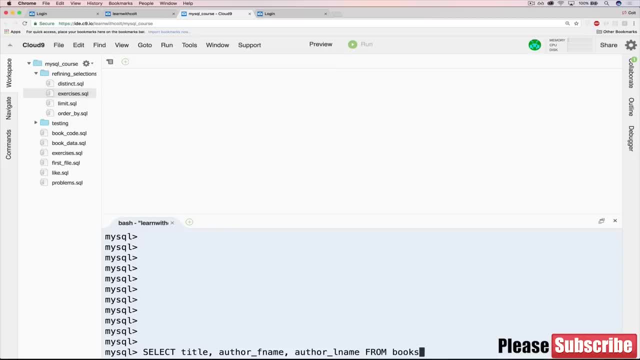 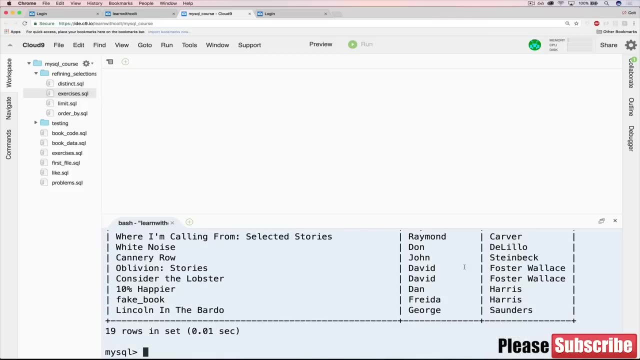 answer is going to have count as the second type of name. like washout and give together, we can see the number. that tell us the number by narrating and string or anything like that- yet So we have a much bigger data set. right, Let's do a group by now. 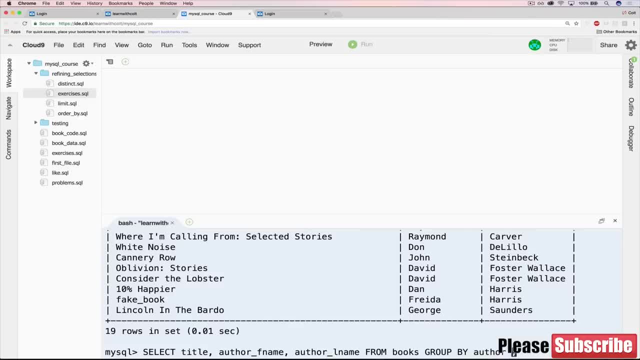 Group by and we'll do author last name And we're going to just do the exact same thing. I want to know how many books each author has written And we will run into problems. I'm just telling you now with this Harris right, Because we have two different Harris's: Frida Harris and Dan Harris. 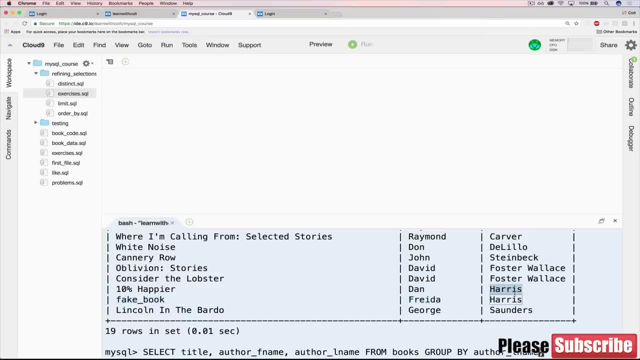 But when we group by last name, it just treats them as one. So it will say Harris has two books, which technically is true. The last name, Harris has two books. Okay, so if we do this and just hit enter, it's not useful. I don't know why you would ever do that. honestly, It just is giving. 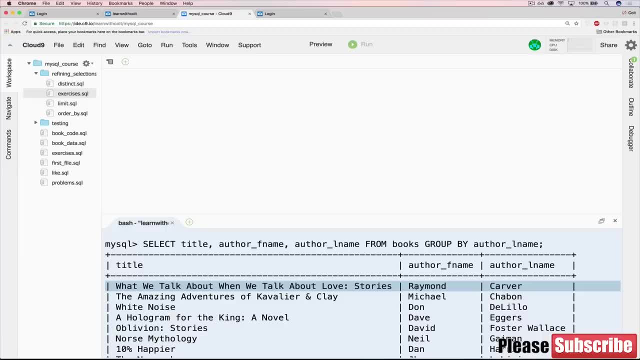 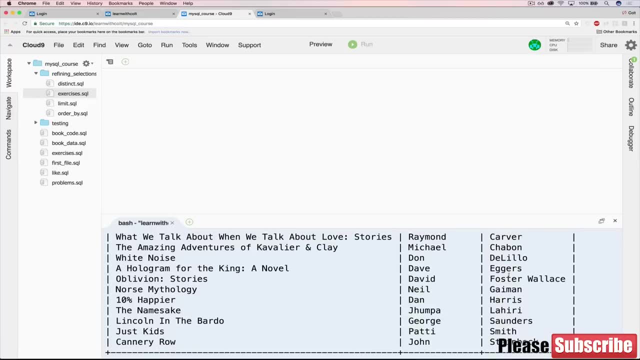 you sort of a preview of the mega rows, if you will. Basically, it's just taking the first book by Carver, the first book by Harris, but we don't see how they're actually grouped. So it's not that useful. It's not useful. 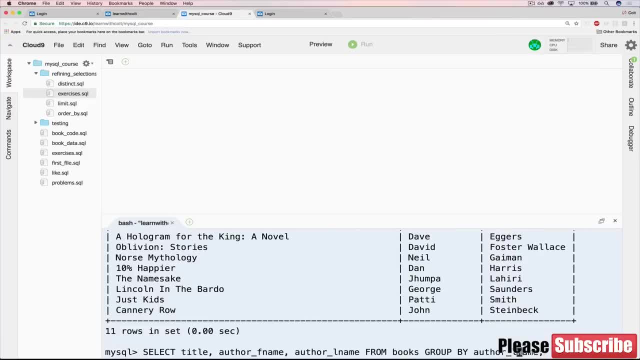 It's not useful at all, honestly. So what we want to do is, rather than just title, author first name, author last name, let's do count star And remember: count star in this case is referring to the grouped rows. So it's going to go to each of those grouped rows and count how many rows have. 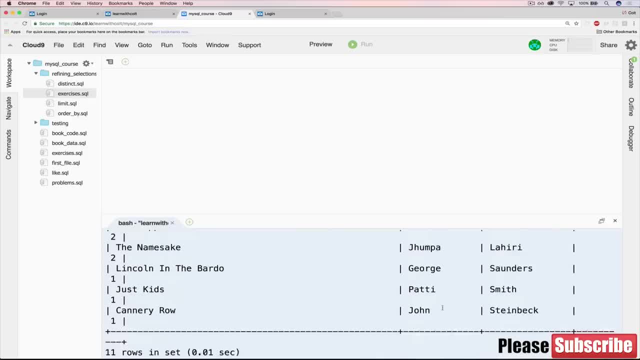 been grouped together. Oh, and this is kind of a mess to look at. So let's actually get rid of title. Let's just do author first name and last name. Now we can see. So Raymond Carver has two Don. 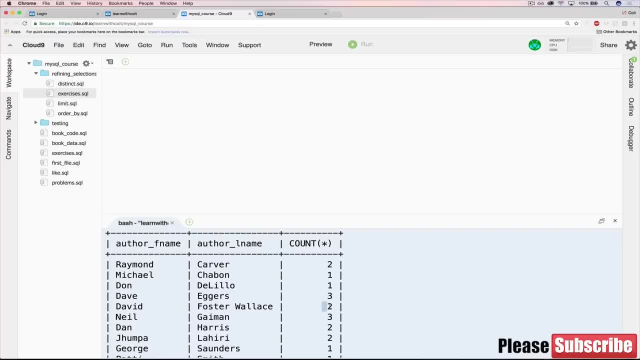 DeLillo has one, Dave Eggers has three, David Foster-Wallace has two, And then, as I mentioned, we have this problem with Harris, because it says Dan Harris has two, but that's not true. Dan Harris has one book, Frida Harris has one book. So to get around that, of course we can do the 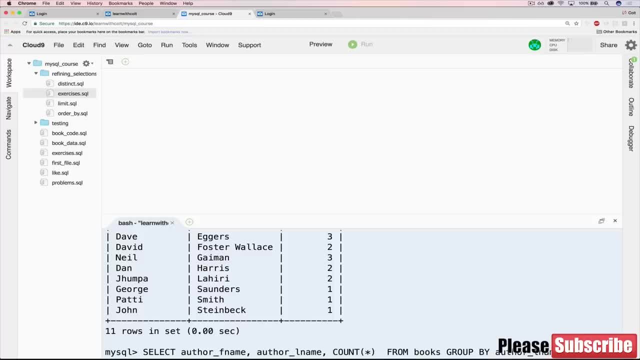 same thing where, rather than just doing group by author L name- hopefully you've seen that this is something that's kind of standardized across MySQL- we can do author F name as well, So it will group where both of these are unique. So then we do. 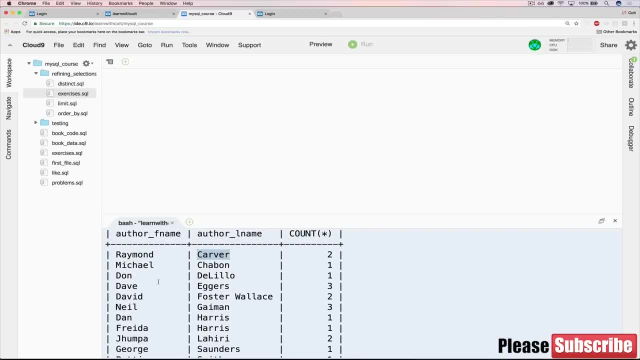 that Everything else is the same. Raymond Carver has two, Dave Eggers has three, Foster-Wallace has two, But if we go down here, we now have Dan Harris with one and Frida Harris with one. All right, So. 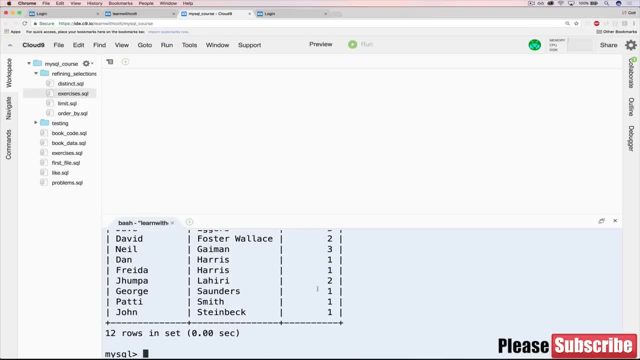 just to show you another thing that we could do. we could also group by released year, So, and we could group by title, of course, but we don't have any books that have the same title, But we do have a couple books that have the same year. So let's say we wanted to get a nice printout that shows us. 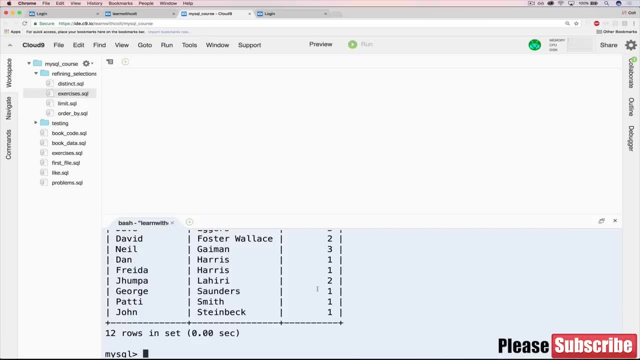 in 2017, one book was released In 2016,. two books or however many books were released. So we can do that pretty easily with just a select And let's do released year comma count star. So if we just do select released year from book, 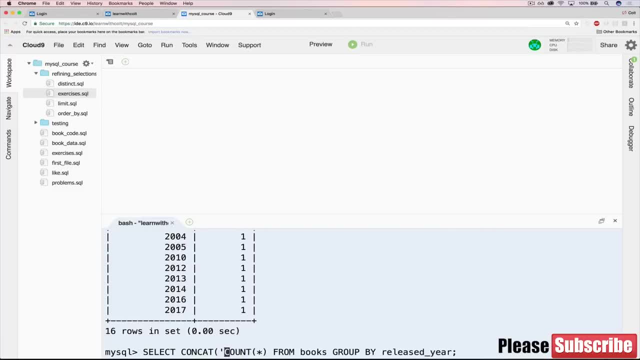 you know, you can see where's the example, I think 2003,. we've got at least two 2003s And I know there's a couple more. I hope there's a couple more. So let's say we wanted to condense. 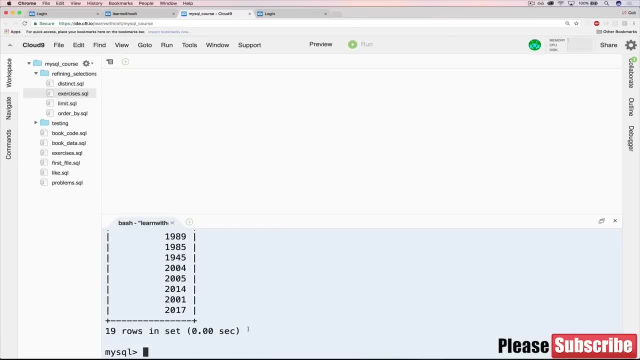 them all together and then put a count next to it as well. We would do that just like this: Select released year from books. We would group by released year Rather than only selecting the release year, We also want to select count star. Let's hit enter. 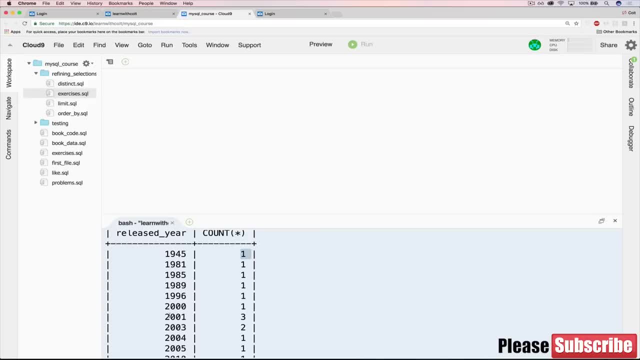 Now you can see we've got 1945, one book. 2001, there were actually three releases. 2003, there were two releases. So you can see that it's working. and if we want to get really fancy, Go ahead. move on to the next video if you'd like, but I'm just gonna show if we want to get fancy and print it out. 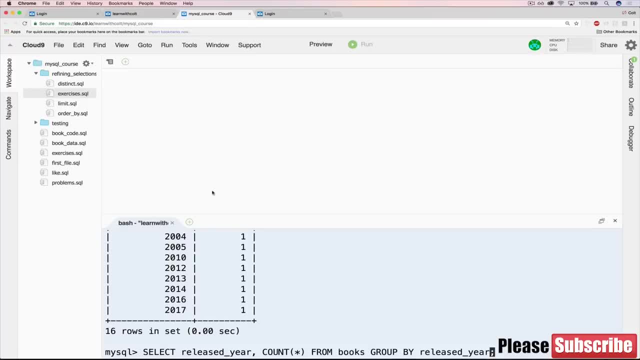 Nicely, we can combine it with the concatenation. We could do something like this: So, rather than just selecting the count, We could do: Let's see a select can cat and we're gonna concatenate the released year Comma. so Let's do, actually, let's add a string before. so I'd like it to say like: in 2010, two books released in 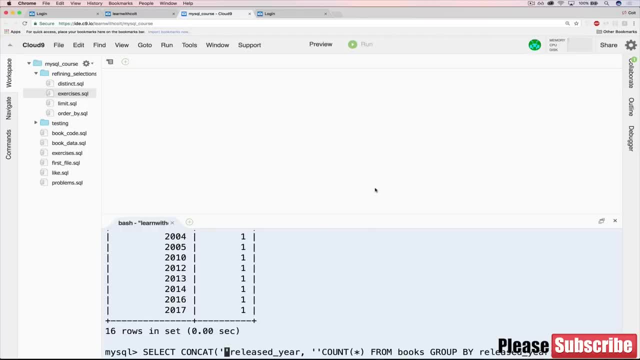 one book. I guess In 2001 three books released. I actually want that string so we can do in the released year, Comma The count, Comma Books released and Technically, just to make sure, let's add parentheses around the s because there's in a lot of cases one book. 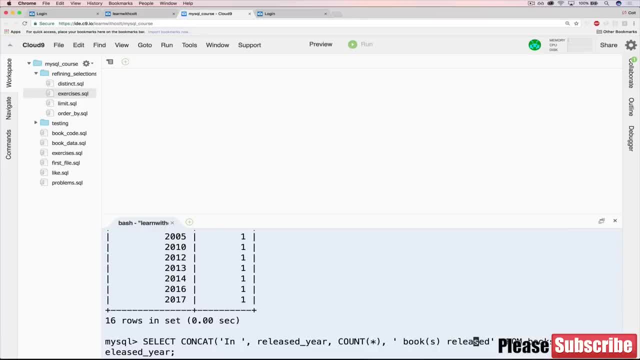 Release. so I don't want to say one books anyways. so let's make sure we have our correct parenthesis here. select the concatenation of in the released year. We probably want to space there, Don't we? this is where it gets kind of annoying that we're not using a separate file. so in 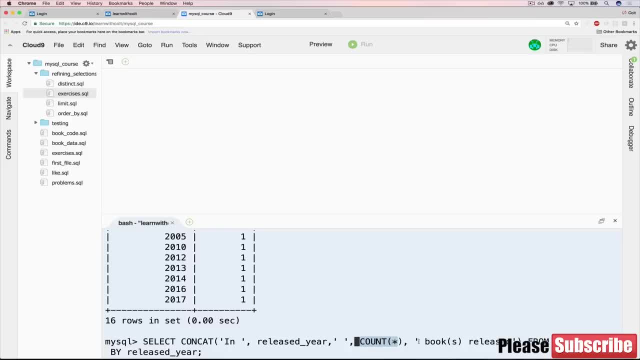 2001, let's say space, three space books released and then, Lastly, to clean this whole thing up, Let's add an add, And we'll just call this as Let's just say year or something silly. We hit enter And we get this nice little table. in 1945, one book released in: 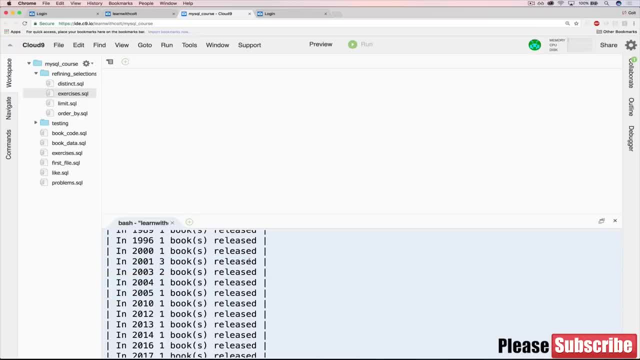 2003: two books released. in 2001, three books released. Okay, So that's it for now at least, with group by. we're gonna be working with it in every video from here on out. in this section, Like I said, we're gonna move on to things like min and max. 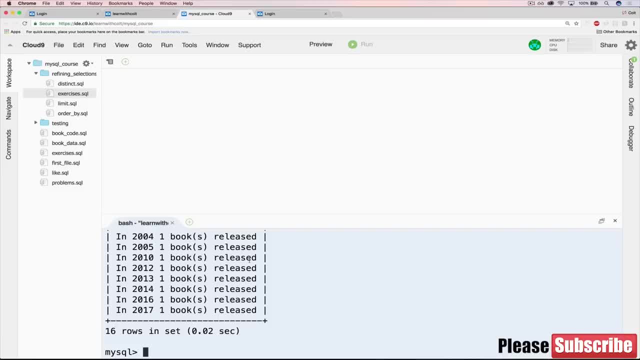 average some fun things, Hopefully sort of fun. Congratulations if you made it through this video. like I said, it's a little bit weird. It's different than what we've done before. Hopefully it wasn't too boring, Okay. So next up we're going to continue on with two new functions and they go together. 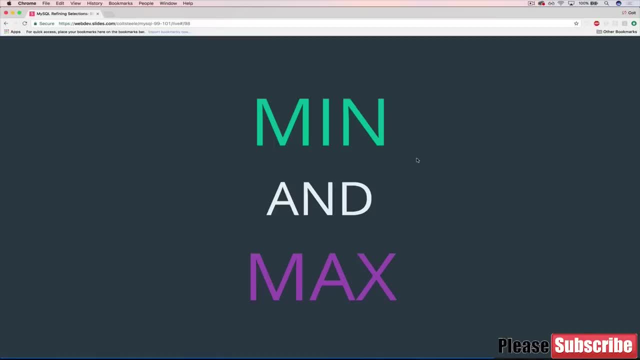 They fit well. They're min and max, minimum and maximum, and they do what they sound like, what their name says. They help you find and identify minimum values in a table or maximum values in a table, and we can use them on their own and We can also combine them with group by to get further insights. So we're gonna see how to do both. 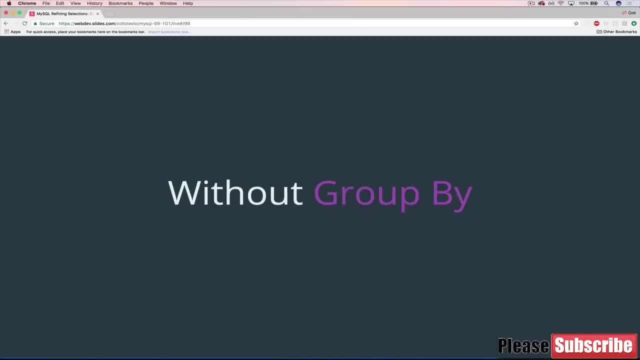 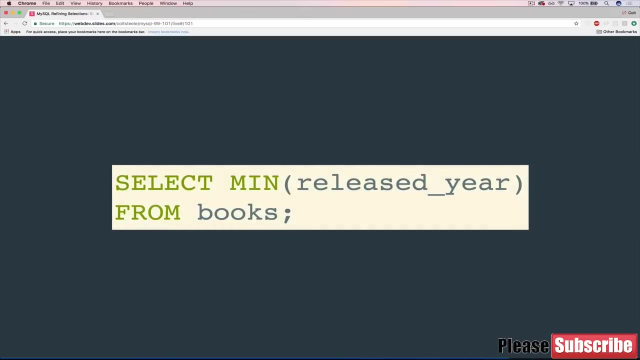 We're gonna start off by using min and max without group by, So we can do things like find the minimum release year in our entire table, So you know what was the first year any book was released. and to do that just looks like this: select min. 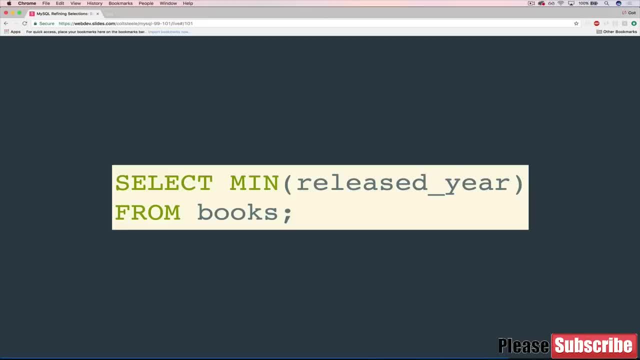 Release year in parentheses from books. So, Just like we did with Count, where you could just count all the books if you wanted to, you can just use min on its own. So let me show you how to do that. Now go over to cloud 9 and we can just do a select min. 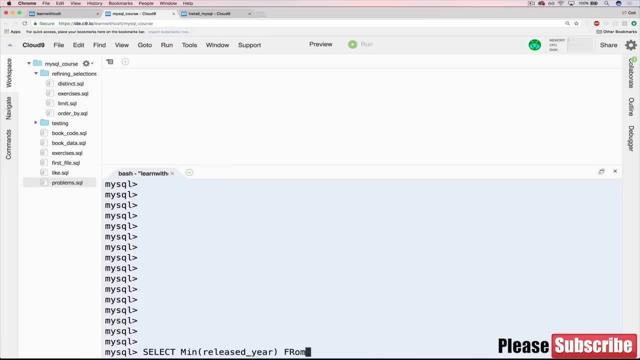 released year from books, and 1945 is the earliest book that we have released, the earliest year that a book was released. We can also do something like select min pages if we want to see what's the shortest number of pages. and That's that tells us: 176 is the shortest. 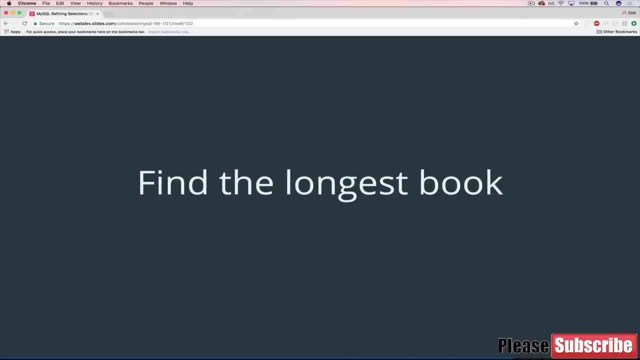 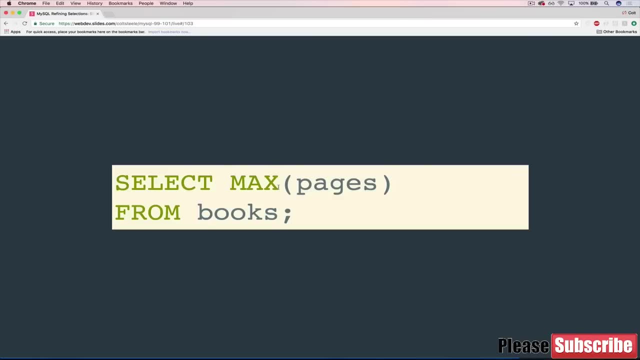 so of course, Maximum works the same way. So instead of min, we just type max and my X, and it does the same thing. So here we're finding it. Well, it doesn't do the same thing, It works in the same way, but it does the exact opposite. 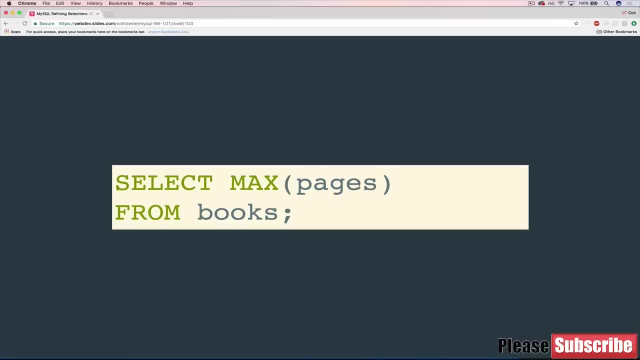 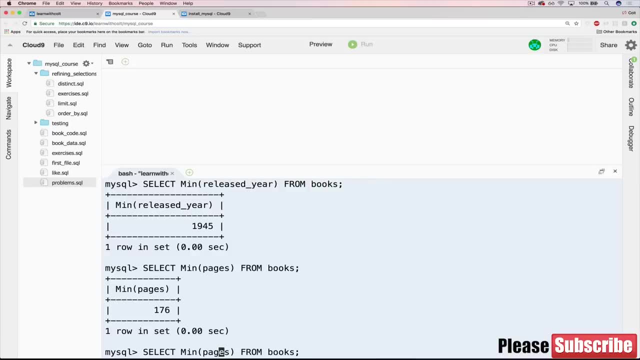 It's going to tell us a return The longest or the highest number of pages. So if we do that, I'll just recall that last line and just change it to be max 634. that is our longest book, and we could do the same thing with year if we wanted to. 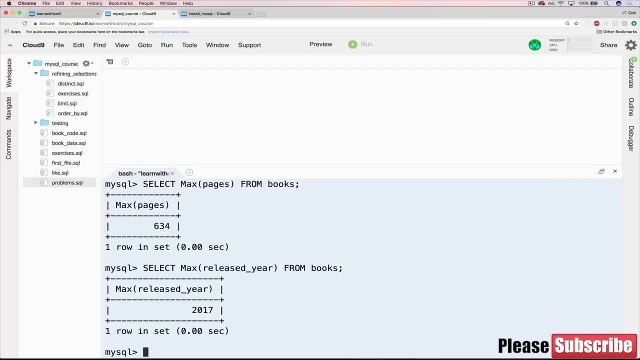 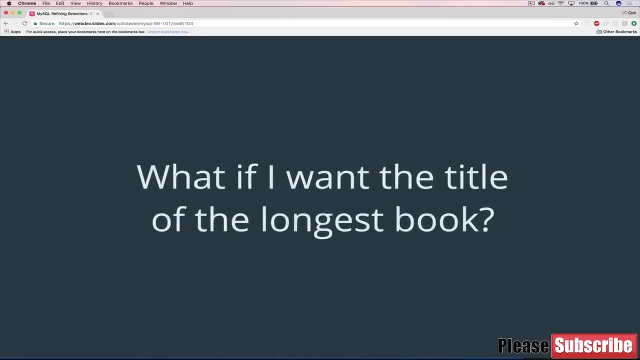 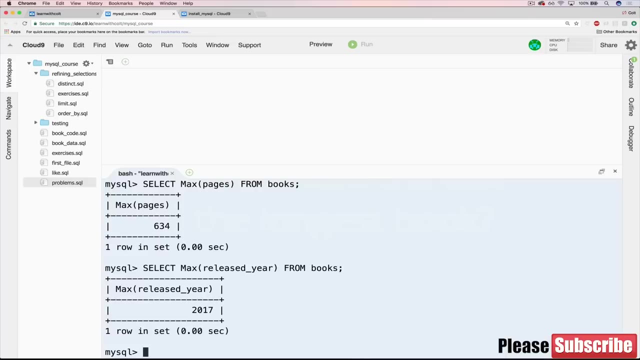 2017 is our most recent year. It's the highest number year. So that's the very basics of max and min, Or min and max, however you want to say it. I do want to call your attention to Something sort of weird. What if I wanted to get the title of the longest book, not just the number of pages, like we have here? 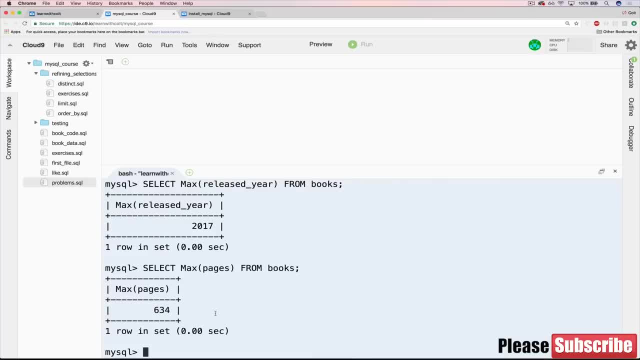 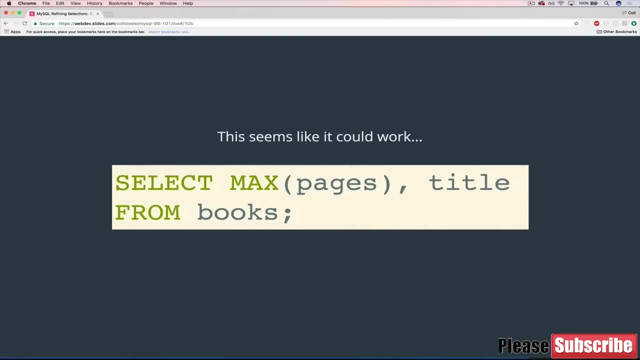 Just finding out that 634 is the longest isn't that useful. What if I wanted to know what is the book, What's the title, who wrote it, The year is released, any other information? Well, you might think you could do this: Select max pages, comma, title from books and, if we try it out, select 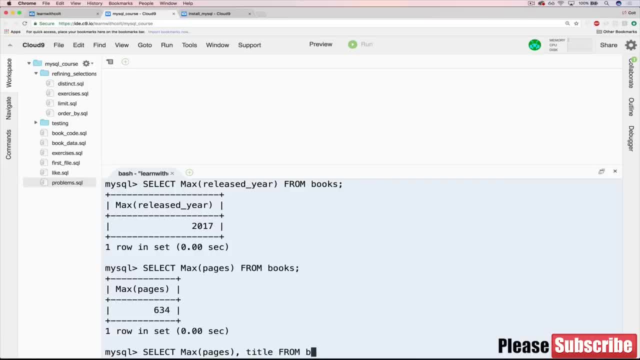 max pages: comma title from books. It says that the namesake is our longest book and it has 634 pages. and while, yes, 634 is the maximum pages in our entire database, the namesake is not 634 pages and, in fact, if we Just do a select and let's just do title: comma pages from books. 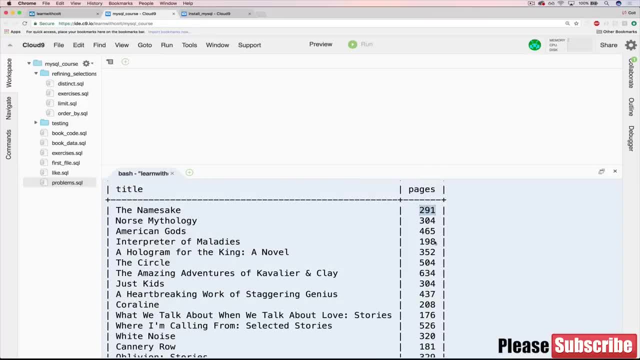 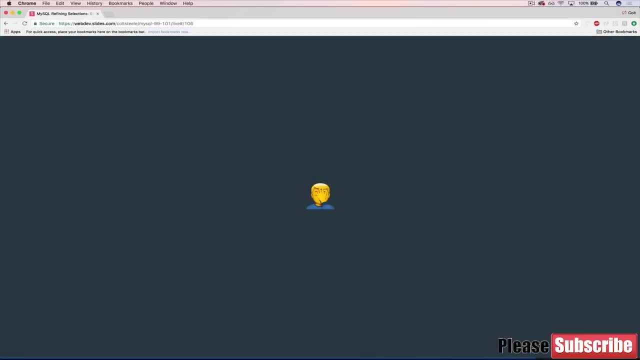 If we find the namesake, you'll see that it's 291 pages, and the one that is 634 is the amazing adventures of Cavalier and Clay. So that's a problem. Here's a nice little graphic I made. It's the largest emoji that I could make on these slides. for some reason, 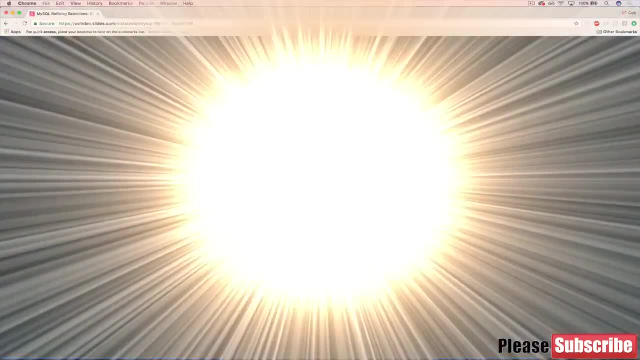 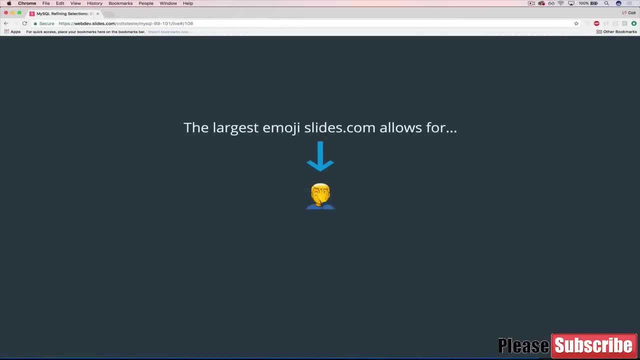 So I'm just gonna go ahead and insert a much larger one now. post production: very fancy. So how? how do we get around this? There has to be a way, and in fact, there's multiple ways in the next video. It's a bit of a cliffhanger here. in the next video, We're gonna see a couple options. 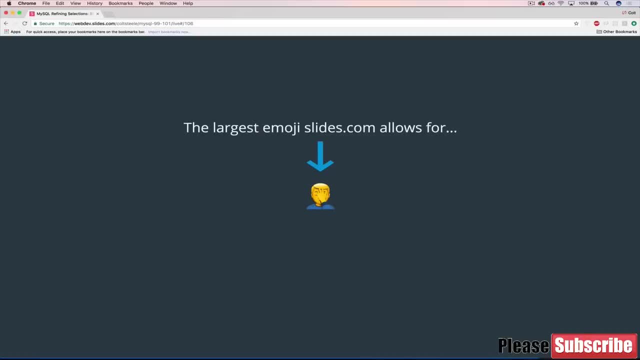 Including a preview of a more advanced method, something that we haven't seen just yet, But there is a way to do it, using what we already know, Something we learned a couple of videos ago. All right, Next video. Okay, So what we're discussing in this video- in case you didn't see the last video that leads into this- is: 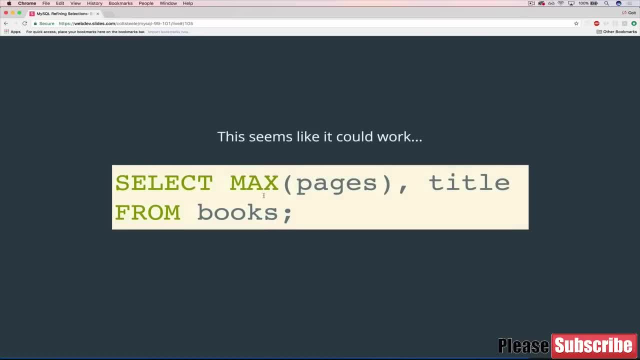 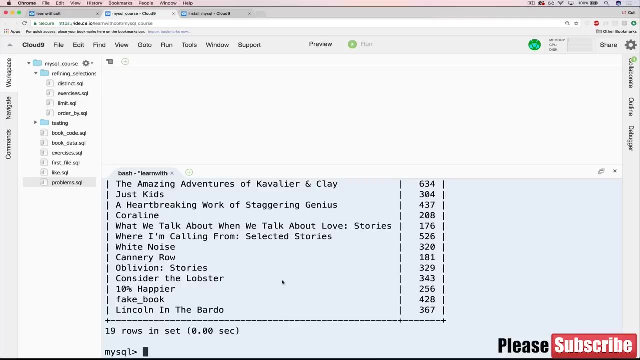 That there is a problem With trying to do something like this: select max pages, comma title from books. If I want to find the title and the, or find the title of the longest book or any other information along with the maximum pages. It doesn't work And what it's doing right now is actually returning. 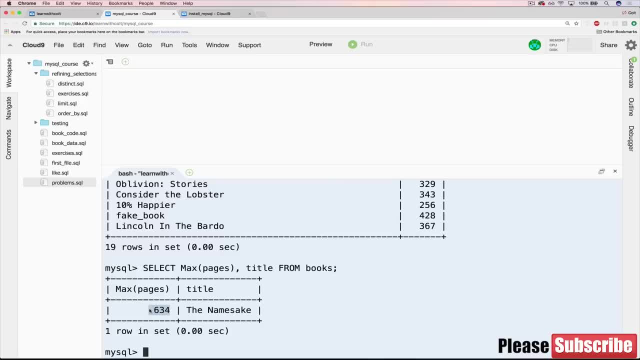 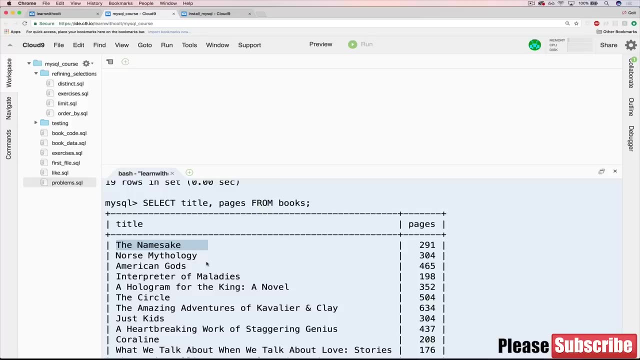 Oops, here we go is first finding the longest pages- maximum pages, which is indeed 634- but then When I asked for title, it's actually just giving me the first title, the namesake and the reason that it does it. it's kind of complicated and weird, but basically you can think of it as: 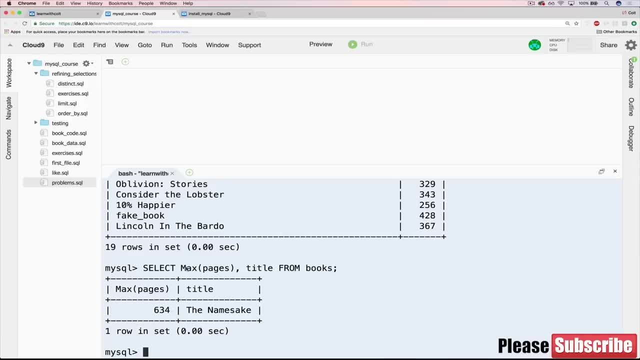 sequel, or mysql, is executing this and It finds the max pages first, which is independent from this, So finds this 634 and there's only one row that it's preparing to print out. so then we get comma title and There's only one Spot to fill, so just takes the first title. So these are independent of one another. They're not connected, unfortunately. 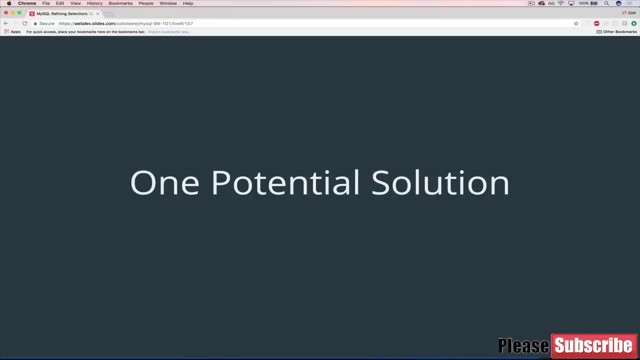 But there are ways around it. So the first thing I'll show you is something a little weird. It's not weird overall, It's just weird to you at this point because we haven't seen this before. it Involves something called a sub query, which we'll return to later on in the course, but I wanted to just preview now and 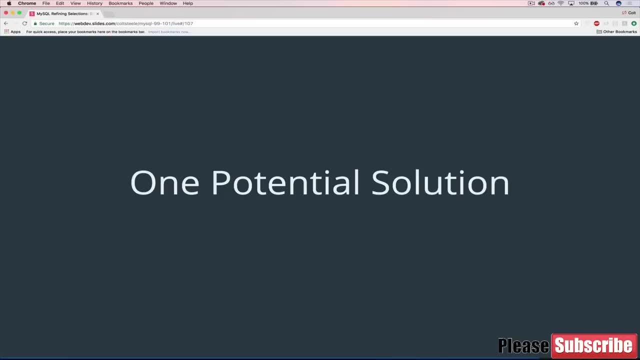 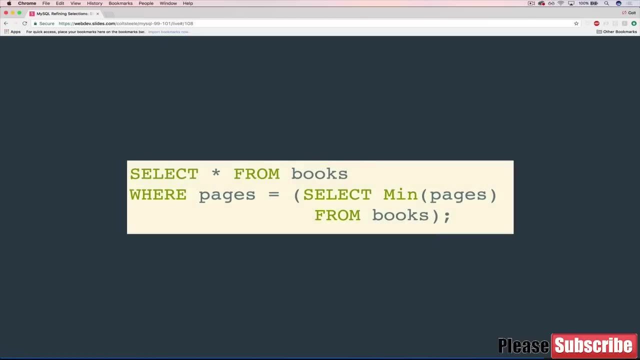 Basically, what it lets us do is run one query inside of another, So it looks like this: Select star, in this case headed start, although we could just do title, but select star from books Where pages equals. and then- this is the weird part- Parentheses. and inside the parentheses We have another query: select- in this case I did min pages from books. 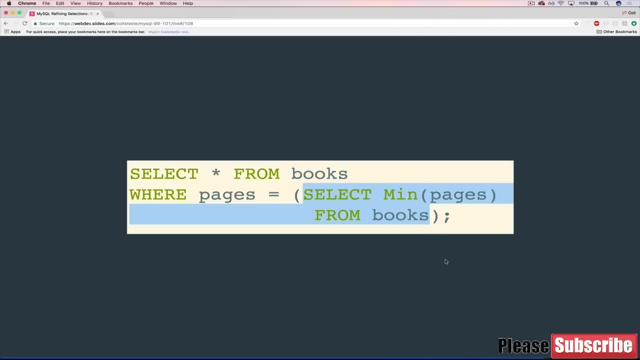 So what's going to happen is that this will actually execute first select whatever we have here. so let's say, min pages, I believe, is 129, or in our case, max pages would be 634, so it's going to find that in return, 634 here, and then this will run: select star from. 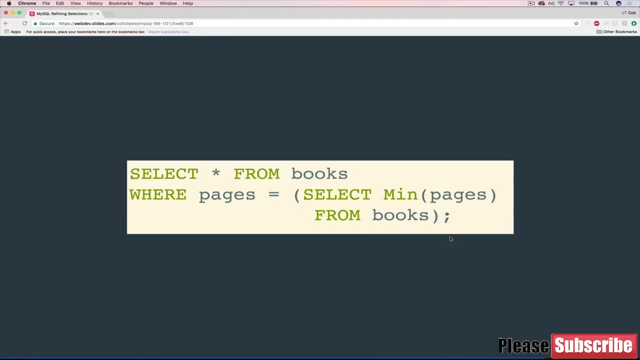 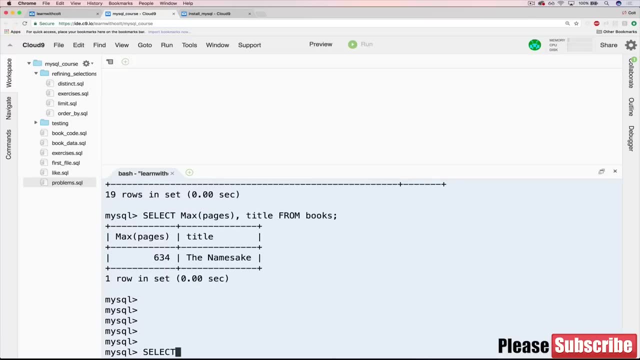 books where pages equals 634. so let's try it out now and I'll show you basically manually what's happening. so think of it as doing a select max pages from books just like this, which is 634, and then copy that and do a select and let's do a- I will do star- select star from books where pages 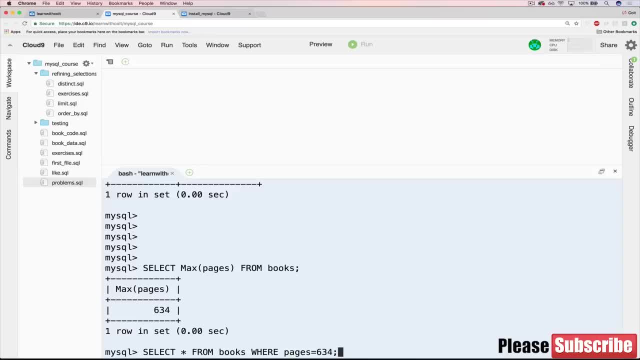 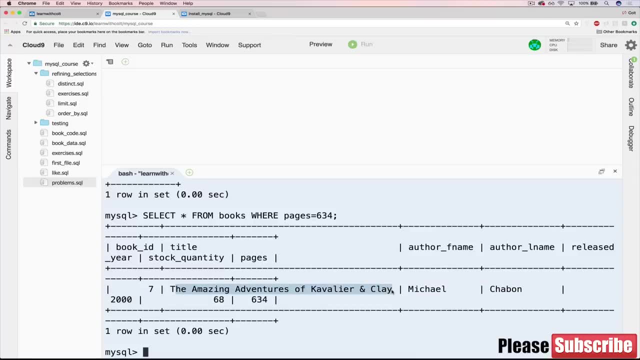 equals 634. so it's a two-step process and you can see, even though our formatting is a little screwed up, we get the amazing adventures of Cavalier and Clay, which is indeed the longest book- 634 pages- so we can do that all at once, or 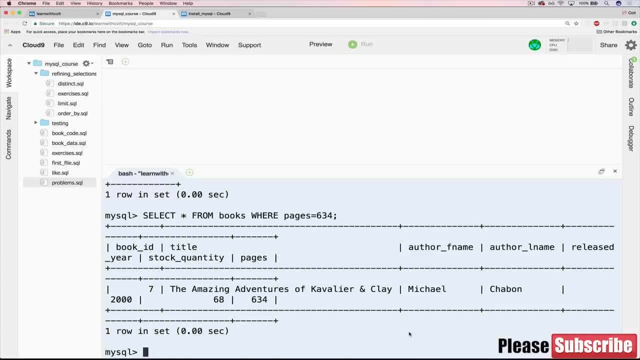 at least in one line of code with: uh, if we just recall this, select max pages from books. that will be our sub query, and so that's kind of going to be a fill in the blank. so we'll have a select and let's just do title and pages. 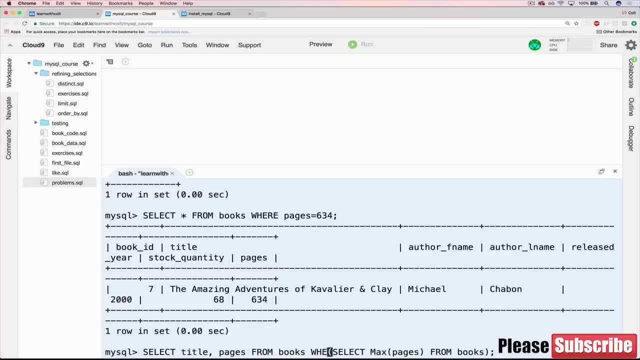 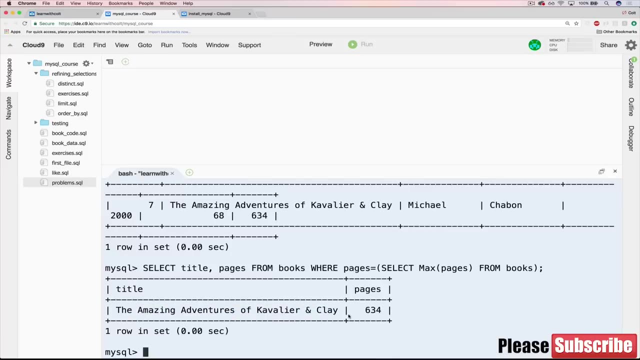 Angst Time from books where pages equals the result of finding the max pages. so it's doing what we just did, but in one line of code, and now you can see we get the amazing adventures of Cavalier and Clay- 634 pages. so we could also do that with Min. and if we just replace this, 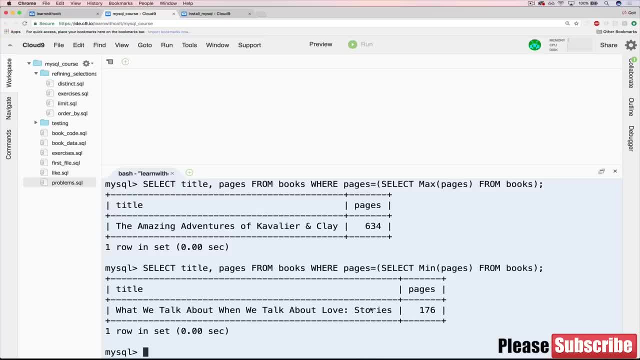 you'll see that Raymond Carver is what we talk about. we talk about love. short story collection: great short story collection, if you like short stories, is the shortest book: 176 pages. so that's all we'll talk about, with sub queries. so that's all i'll. 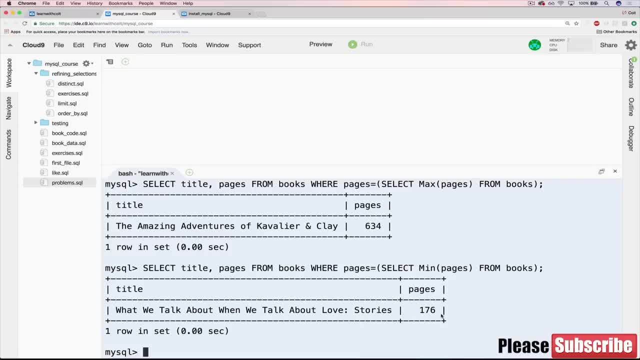 show you, but you can probably imagine there are other uses for them. but there's a small problem. it's not really a problem, but there's something to consider, which is: this is a little bit slow. in our case it's not that slow, it's not slow at all, because we have a very small data set. 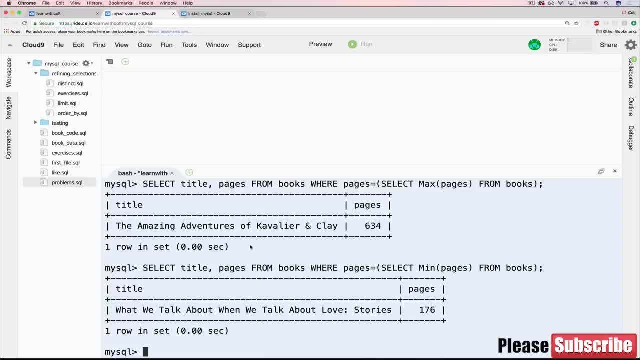 but it's effectively running two queries, so each one of these is run independently. so when we hit enter, when this executes, like i said, two things are happening: two separate queries that are going to take time, each one of them. every time you do a select, it takes time and there's a faster way. 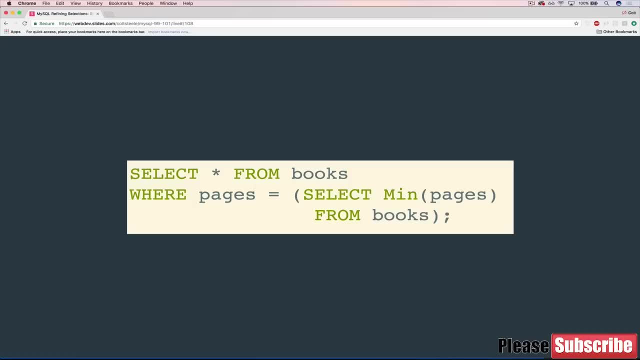 if you are worried about speed, and it involves something we've already seen. so there's nothing new, no fanciness, no top secret. you know advanced features, sub queries or anything like that that you haven't been introduced to yet. there's a way of doing it using what you've already seen. so that way is. 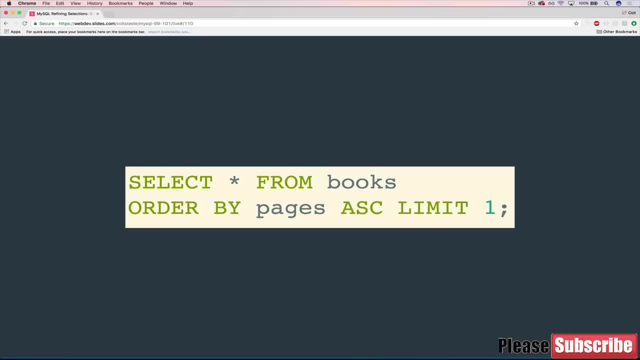 using order by. so what we could do is just order by pages in ascending order. so do a select star from books, order it by pages ascending, and then just limit one. so chop everything else off and just take the first one, and that will give us the exact same result, but it's not going to take as much time. 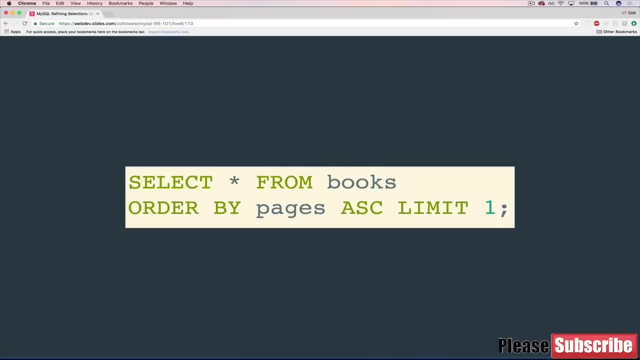 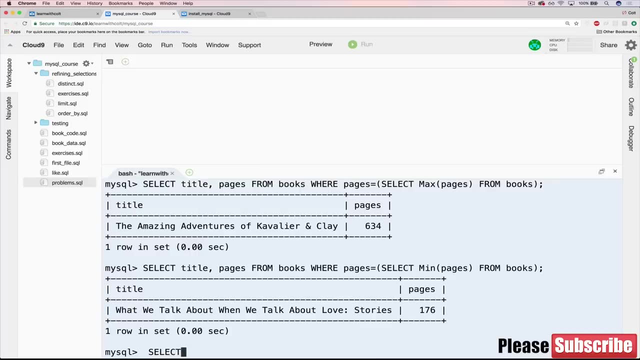 it's not going to be as difficult for my sql to run because it's only selecting one thing and it's only running one query. so let's try that. we'll do a select and let's just do title and pages from books and instead of doing our where pages equals blah, blah, blah, we'll just do our order by. 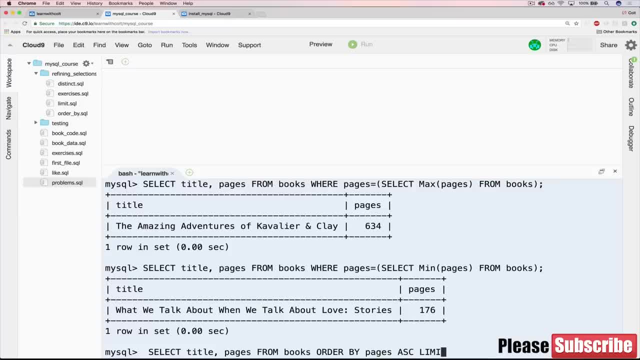 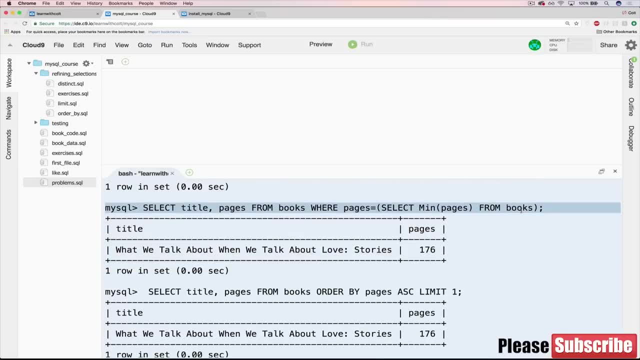 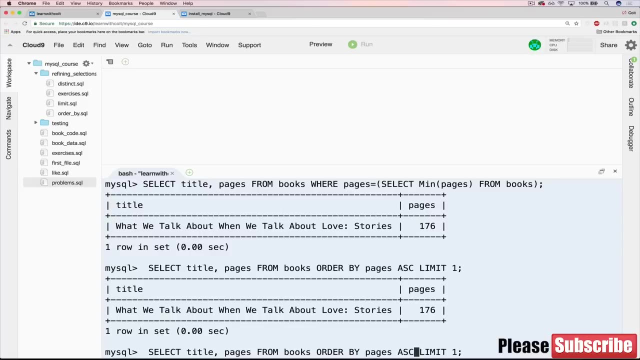 and then we want to order by pages, ascending limit one, and we get the exact same result that we got before with our longer query. that involves a sub query, and we can do the same thing with min. and to do that we just change our order. and yes, it still bothers me: four letters d-e-s-c, but ascending. 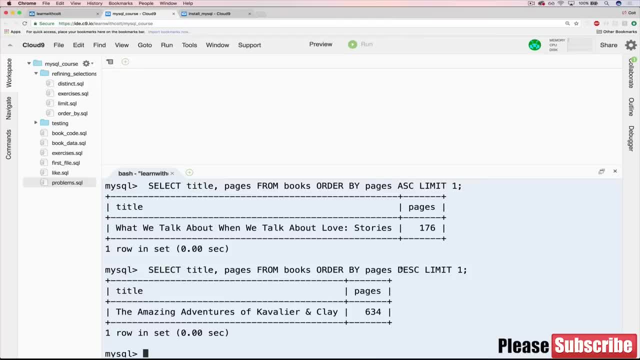 is only three letters, so inconsistent. but if you remember that d-e-s-c for descending, you'll see that the longest book is, yet again, the amazing adventures of cavalier and clay. okay, so that was a bit of a tangent, but it's important to address because i think a lot of people myself 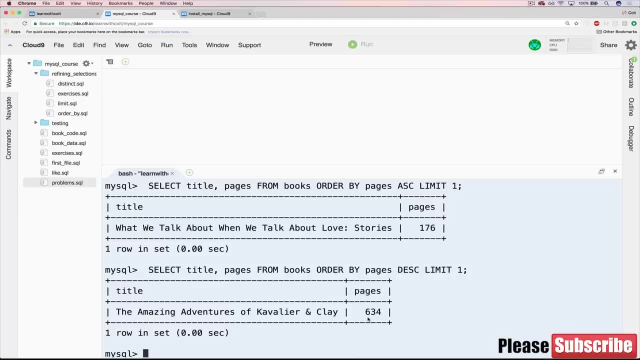 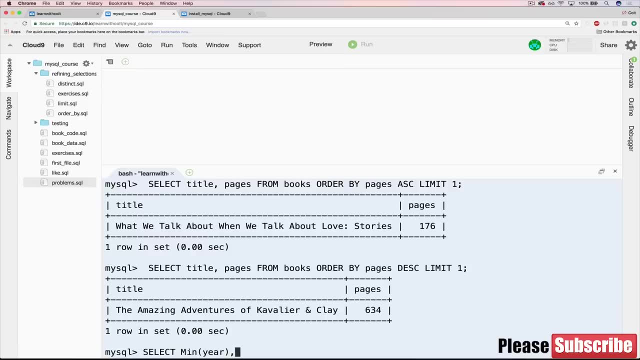 included. i remember when i was learning this stuff, setting out and thinking that you could do something like select min- let's say year, comma, title comma- let's say stock quantity- and that it would go find the minimum year and then the corresponding title instead of stock quantity. and that's not the case. that's just not how it works, as we've seen. 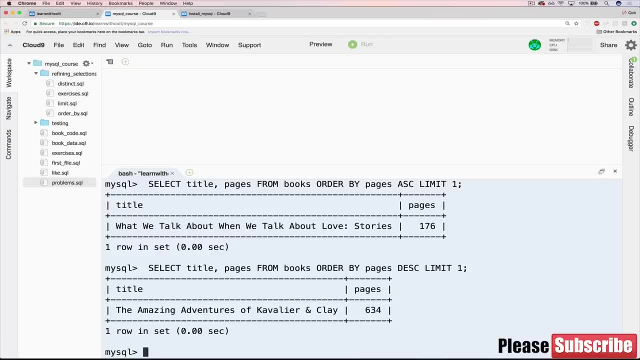 so i just wanted to point that out and highlight a couple of solutions, just so that you're aware, going forward, things aren't always as intuitive as you would hope. okay, next up we're going to continue with min and max and use them in conjunction with group buy. all right, so i 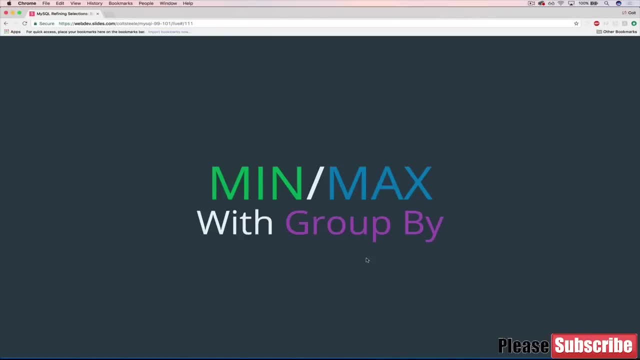 know you've been dying in suspense waiting to see how you use min and max in conjunction with group buy. well, it's finally time. so the way we do it is really similar, identical to how we did count when we use that along with group buy. so let's take an example. 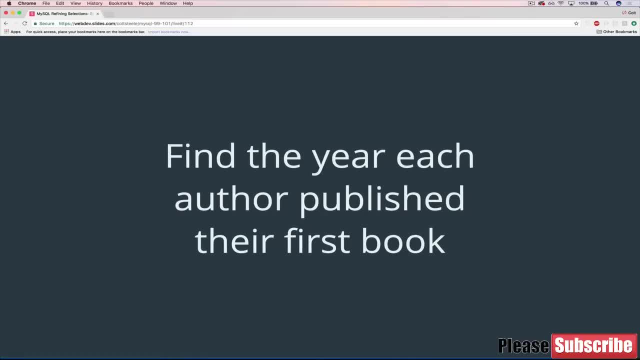 problem. first something like this: find the year that each author published their first book. so we want something like i don't know raymond carver and his i i don't actually know this, but let's say that in our database his first book was published in sometime in the 80s, i believe 1981, let's say, and we want to do the. 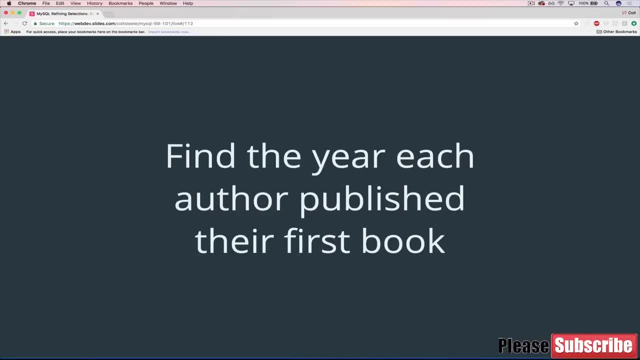 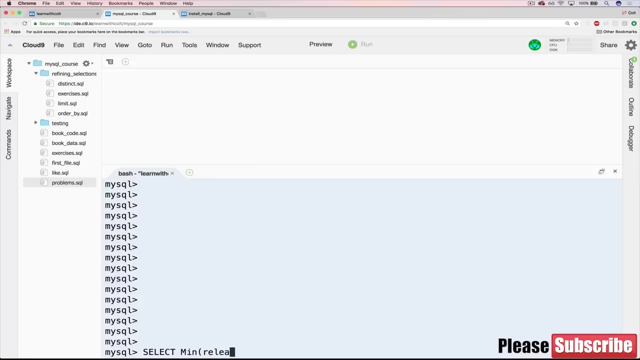 same thing for, let's say, david foster wallace, and his first book in our database was published in 1999 or whatever it is, don't quote me please- and so to do that, basically what we're doing is finding the minimum release year, but we can't just do this right where we do a select min released year. 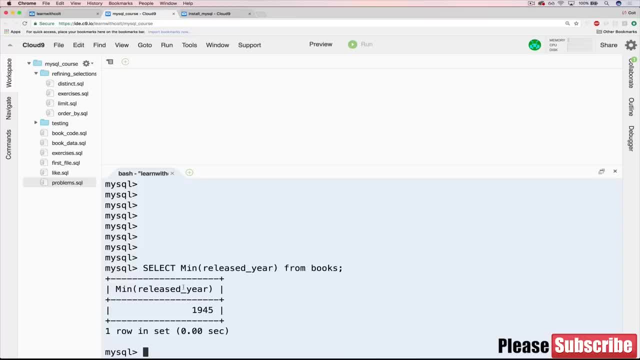 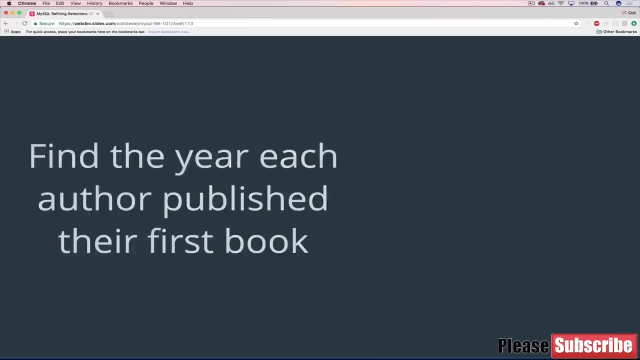 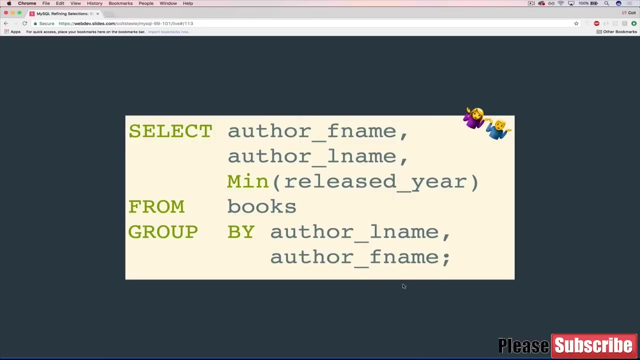 from books because that only gives us the absolute minimum. we want to group all of our books by author, so unique author, and then find the minimum release year for each one of those. so we need to use group by and min and it looks like this and yes, i know it looks kind of long, as this emoji tells you, it might be a little confusing. 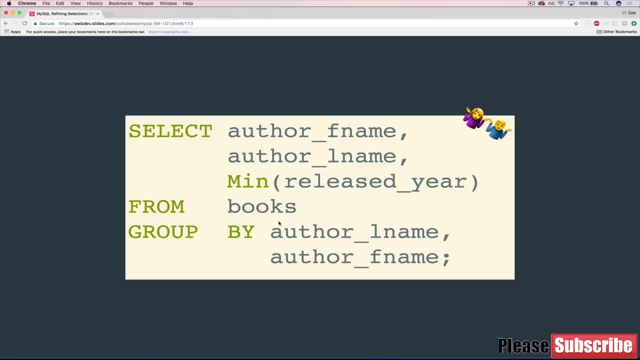 basically, let's focus on the important parts first. which is this right here? and then the group by state. now remember, when we do group by, i'm doing author l name, comma, author f name, because we have two authors who have the same last name and so i don't want. i believe it's frida, harris and dan. 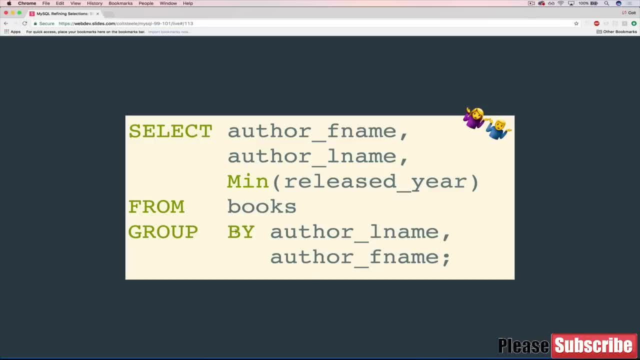 harris, i don't want their books grouped together, so we're separating it out. so this is going to group all of our authors together, make those different groups- i call them what i call them super rows or something like that- and then for each one of those we're going to find the minimum. 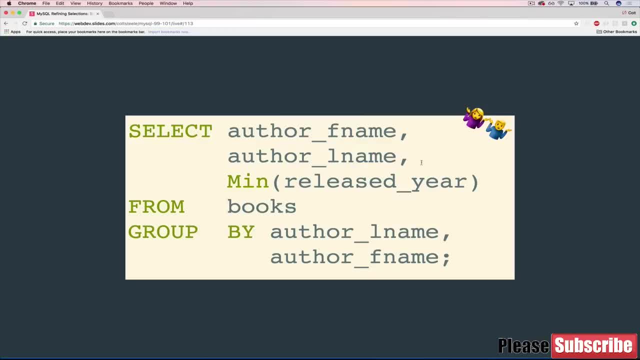 release year, as well as the author first name and last name, because if we just find the minimum release year, it's not that helpful to see if that's all we print out. we want something like raymond carver 1980, rather than just seeing 1980.. so let's give it a shot. 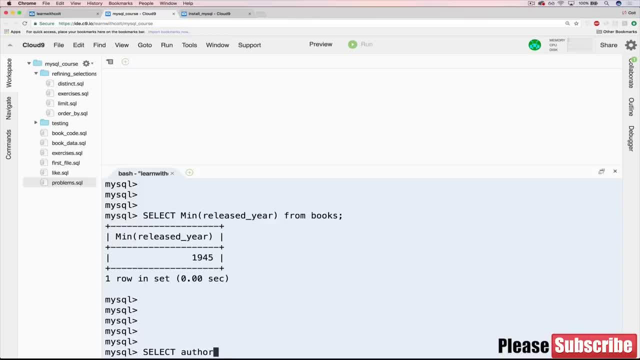 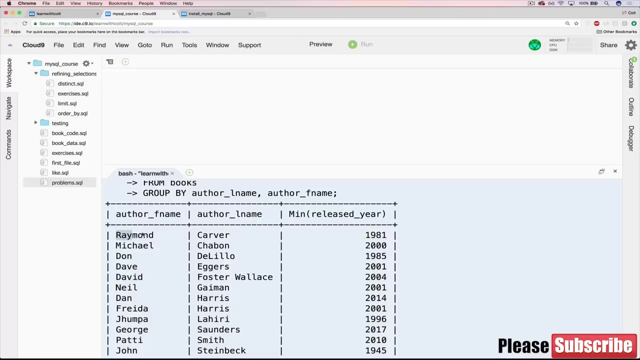 make some space. we'll do a select author f name comma. author l name comma, min released year and then i'll do it on a separate line from books group by. and we want to do that double author l name comma. author f name. let's hit enter, here we go. so we got raymond carver and the minimum. 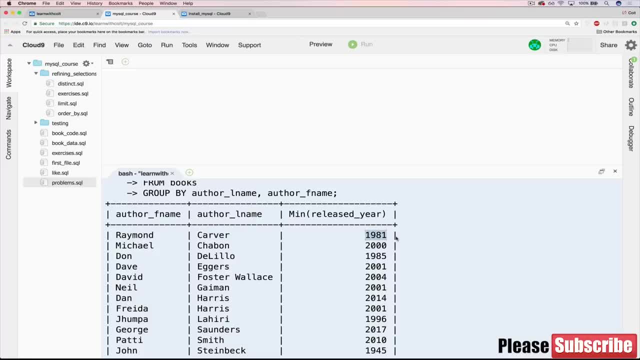 release year for him is 1981, which i think is what i just said, or what i guessed. um don let's say dave eggers, and we've got 2001, david foster, wallace 2004, neil gaiman 2001 and so on. we can see the. 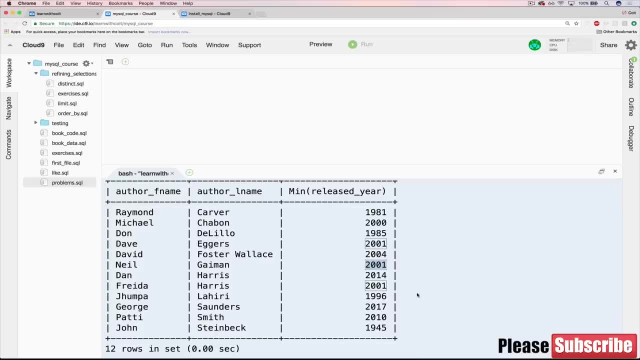 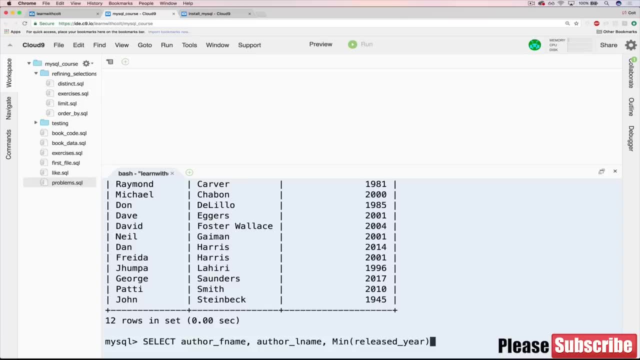 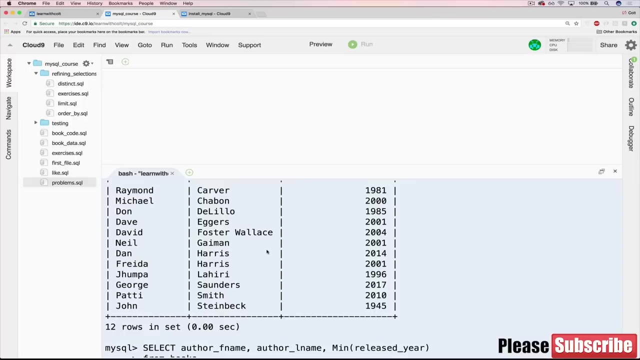 minimum release year for each author and, just to you know, hit this twice. um, oh well, that's annoying by doing it on separate lines. if i had left off here, let me finish this from books group by, and let's just say author l name. if i just left it that everything looks the same except for our two herrises. 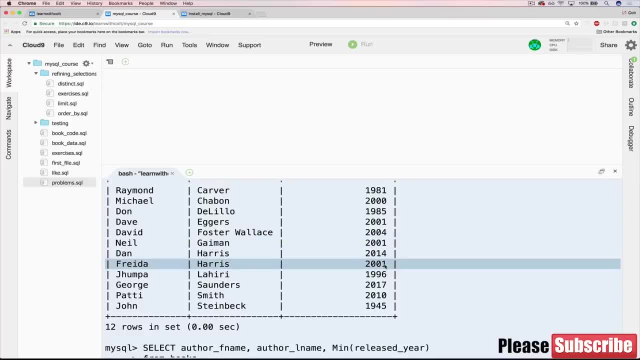 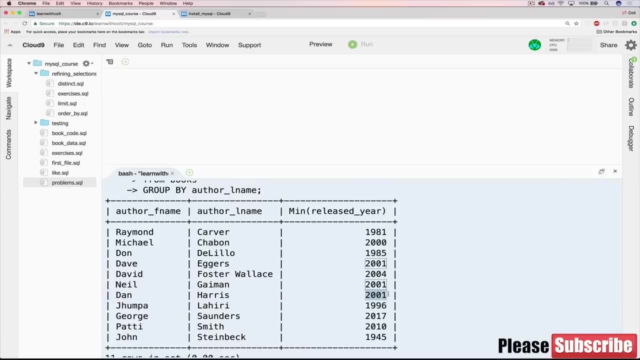 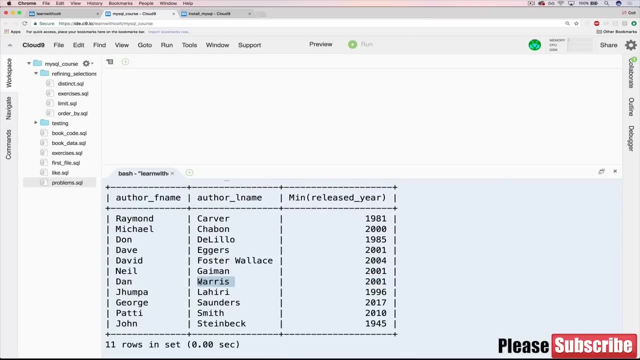 dan harris 2014- frida harris 2001. well, now all we have is dan harris in 2001, which is not true. he never released a book in 2001. uh, frida harris did, and that's because we're grouping everything by harris, and so it puts dan and frida together, so that's why. 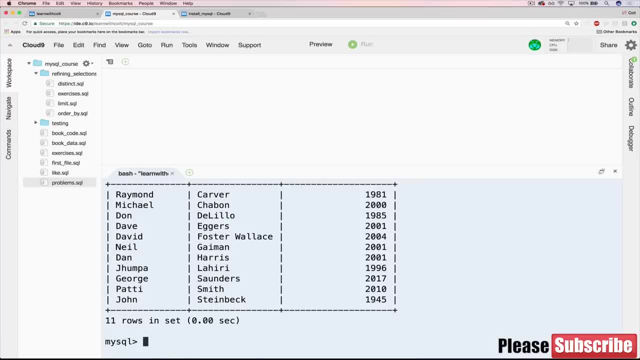 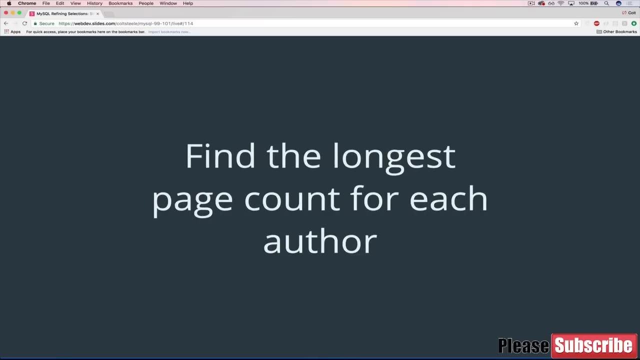 we need both, and so we're going to continue using that group by author, l name, comma for F name- quite a bit as we progress through these group buys and the next couple of videos. okay, so we can also do something like find the longest page count for each author. it's very, very similar. we just need to use max. so 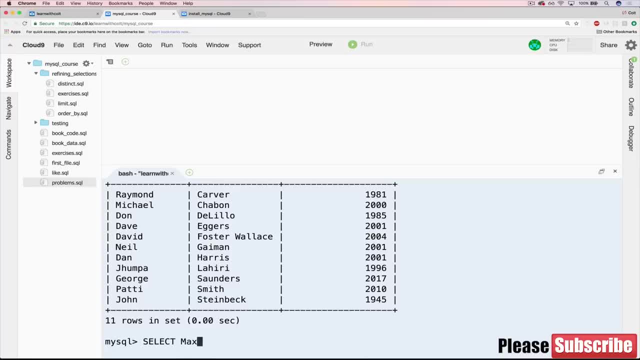 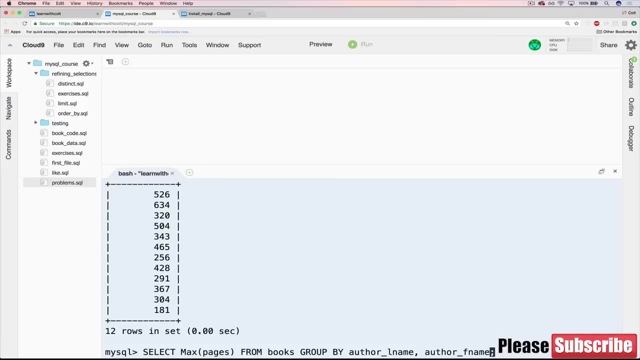 that's going to be a select max pages from books group by: and then our same author L name comma author F name, just like that. however, we just do that and it's not very useful, so let's go and add in select author F name comma author L. 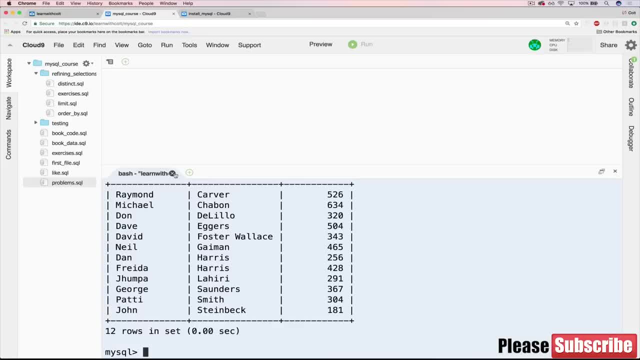 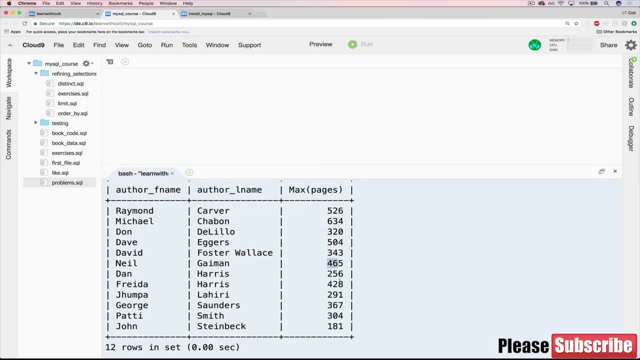 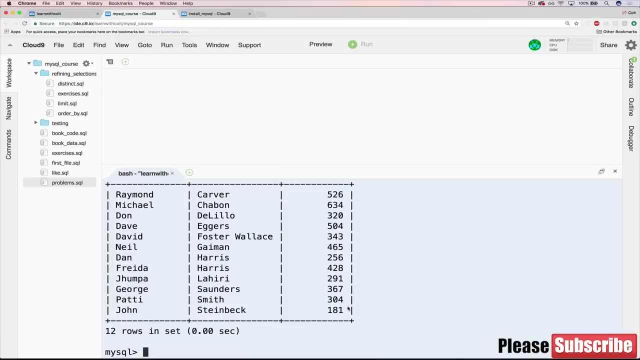 name, comma, max pages. now we can see: Raymond Carver's longest book is 526, Neil Gaiman's is 465, John Steinbeck is 181. he only has one book in there. I believe George Sondheim is 367 is his longest pages. so that's the basics of min and max in conjunction. 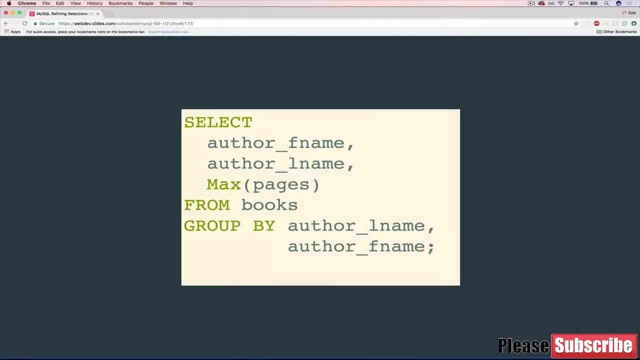 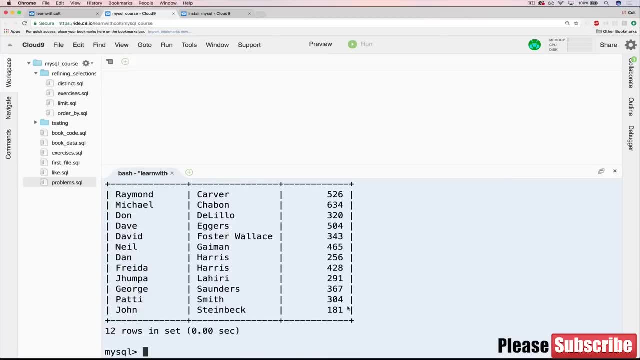 with group by. obviously you could group things differently. we've been doing a lot of grouping based off of authors, but we could group things by the year they were released or I don't know the quantity we have in stock or whatever we have. whatever available pieces of data we could group by, but grouping by author. 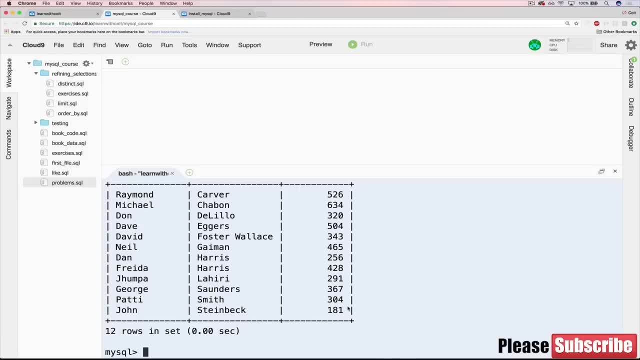 makes a lot of sense for calculating some sort of meaningful data. next up, we're going to go ahead and do a little bit of math and then we're going to continue on with some of these aggregate functions and we're going to, in particular, focus on sum, which will allow us to add things together and average. 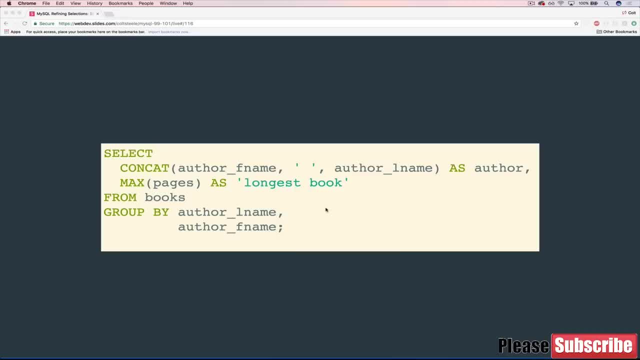 which allows us to calculate averages. oh wait, wait, wait, I forgot I made this slide. I ended the recording and everything started editing and then I remembered I also have this slide here of a nice cleaned up version that just shows you can use things like max and group by along with concat. so all that. 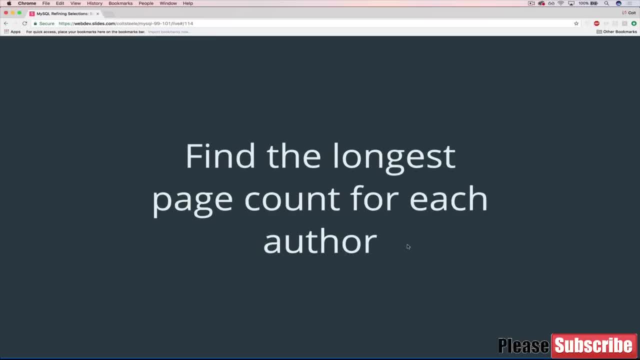 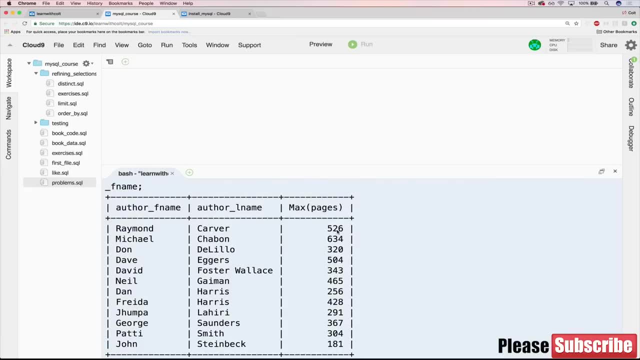 this does is? it's the same thing. it finds the longest page count for each author. but rather than just printing out this mess here- it's not really even a mess, but what it does is it combines some data and it uses aliases so that we have author and 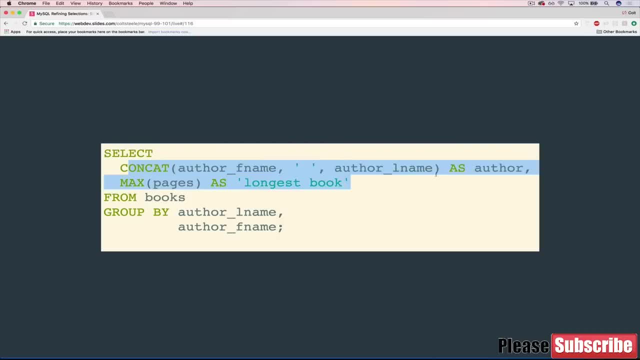 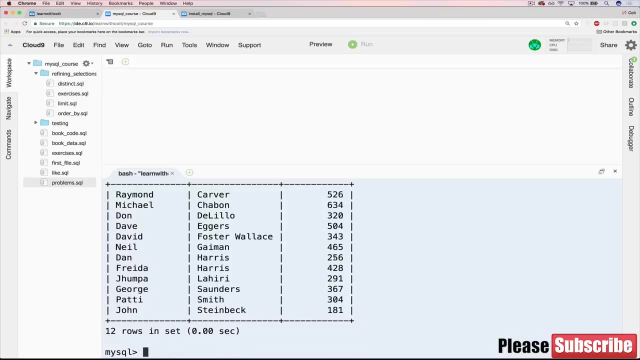 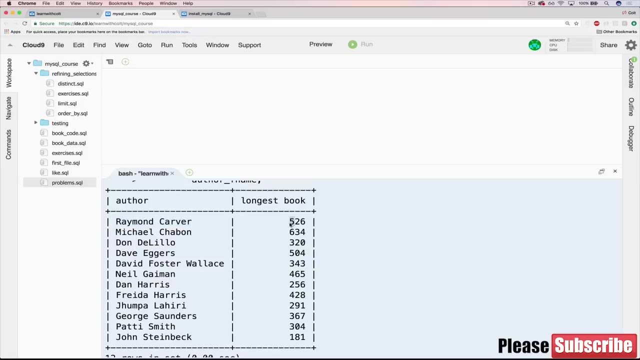 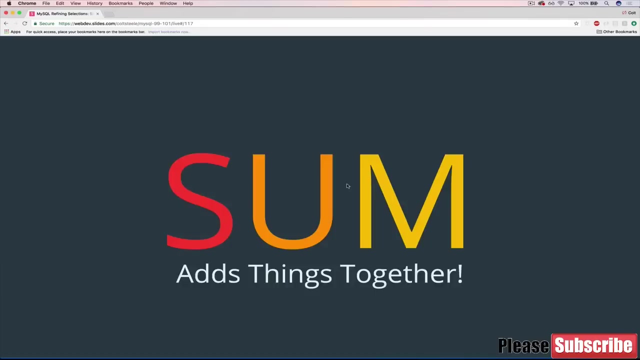 longest book as our column headers and concat, to put together, as you've already seen, the author's full name. so just copy that, run over here, paste it and there we go. we get author longest book and we have a full name here and the longest book. yep, that's it. now we're actually done, I promise. alrighty, then it's a. 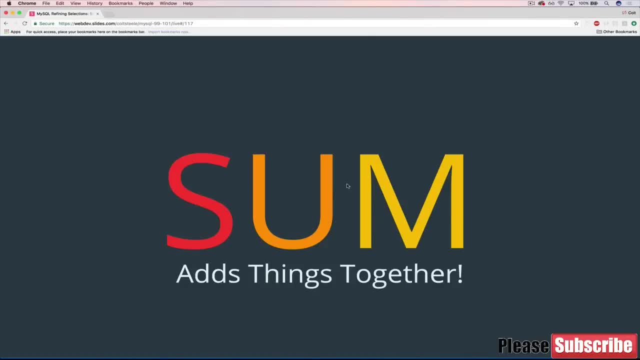 little enthusiastic. ah well, next up we're going to talk about sum, which is another built in function. it does that. it sounds like I know I say that a lot, but it sums together data. it adds things together very exciting. it actually is pretty useful. you can do things like I don't know some together. 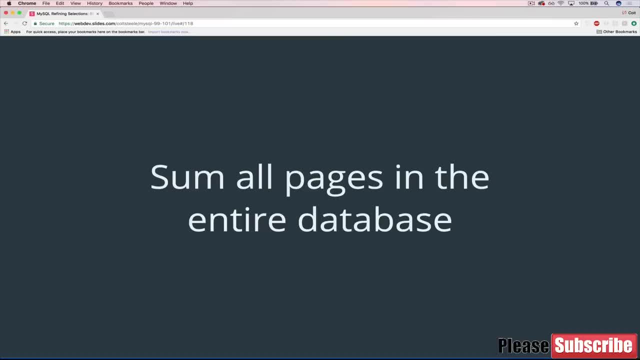 all the profits, all the sales that you've made, or your entire payroll for a given month. let's say you can find some important information using sum, for instance. you might want to sum all the pages in our entire database. so this is following the same pattern as what the last couple videos have. 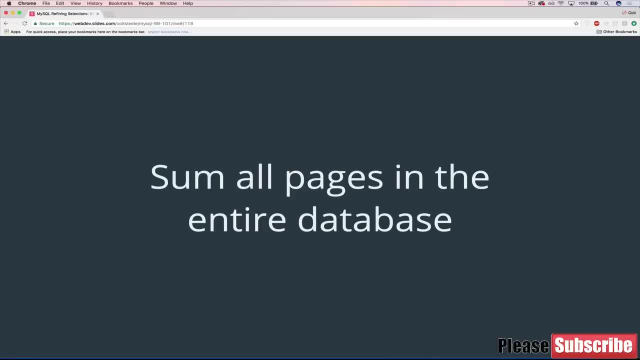 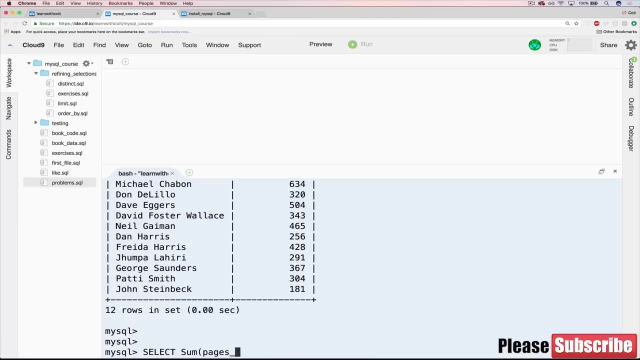 we're going to show you how to use this function on its own, without group by, and then i'll show you at the end of the video how to use it with group by. so okay, sum all the pages in the entire database. it's pretty simple. it's just a select some pages from books and it tells us 6623. 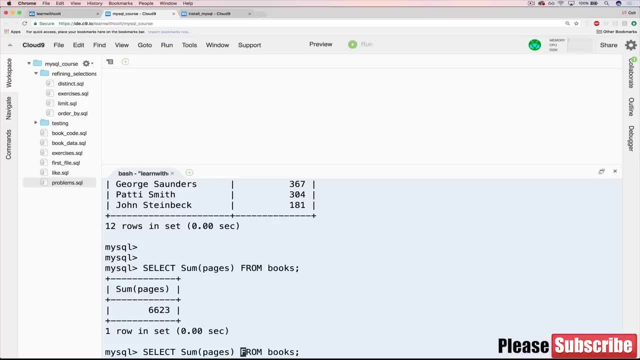 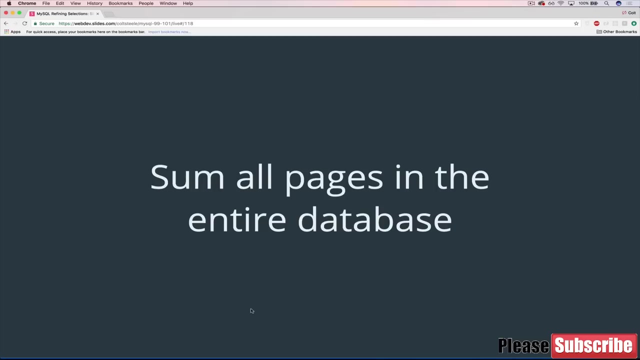 and that's all there is. we could do silly things like some: um, go away, siri. all right, we're back. so we could do something silly like a select some released year. that's just going to add together all the years in our database, let's see 37 996- very important insight we just gained. okay, so that's all there is to summing. 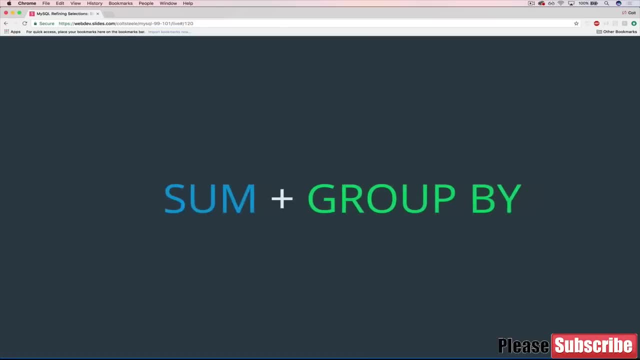 things on its own. now let's see how we use it in conjunction with group by. it works the same way as what we've seen before. basically we group things together by whatever, let's say author or i don't know year, and then we select what we want, and we can use some to help us select. so select. 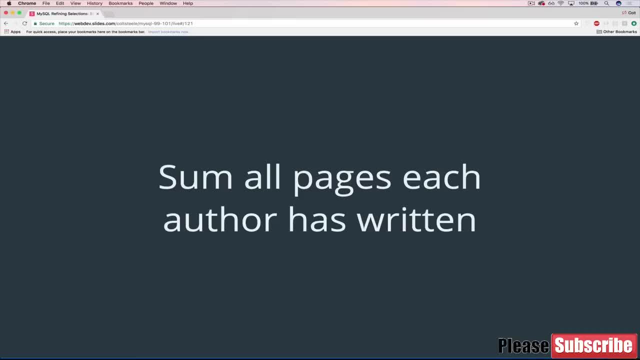 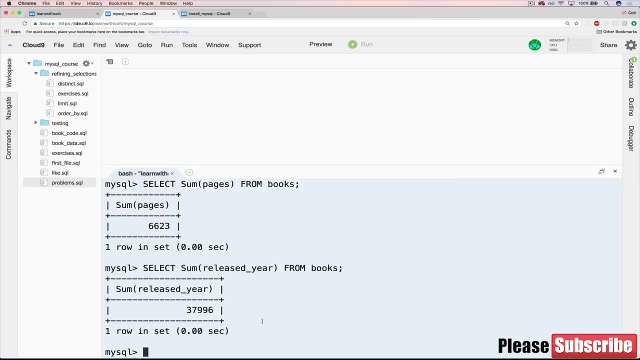 all the pages or sum all the pages each author has written. let's see who, which author cumulative, cumulatively, has written the most number of pages. so we'll start with a select and let's do our the same thing with, uh, with author f name, author l name, and then we'll sum. 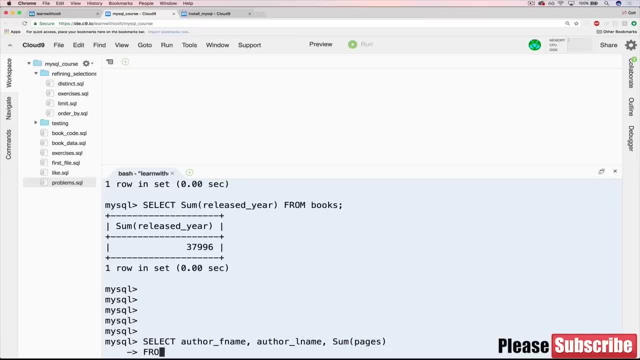 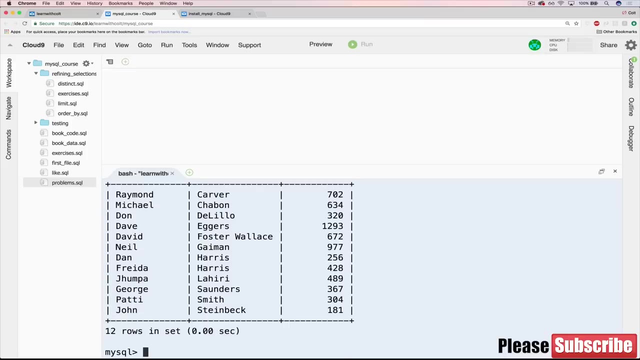 pages. so we'll do that from books. and then we need our all important group by author: f name author. actually we need to do l name first and then f name, just like that you can see, looks like dave eggers has the most 1293.. raymond carver: 702. john steinbeck only has one book, so 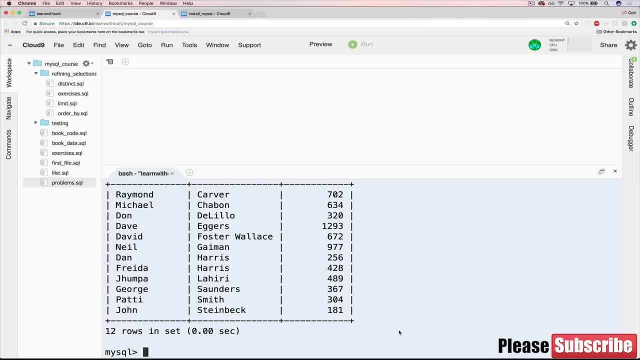 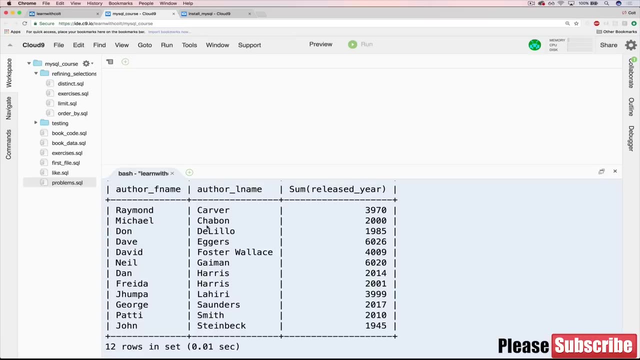 it's only 181 pages and that's pretty much it to sum at this point. uh, we could, of course, do the same thing with, let's say, adding the release year for their books- also a very insightful piece of information that we need, but we can see people who have multiple books, like raymond carver. 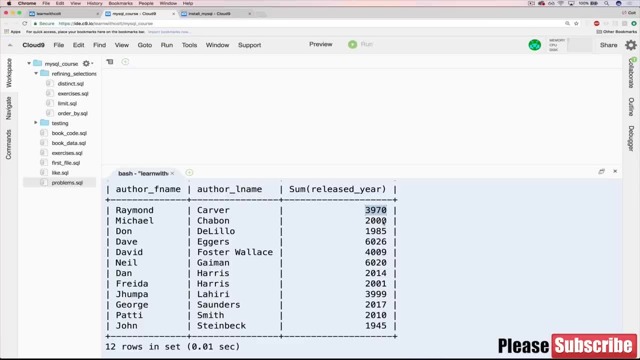 there's multiple years added together. yep, that's pretty much it okay. so that's some. like i said, you may end up using it if you're- i don't know- dealing with sales data, if you're just doing your job and or payroll any sort of information where you're summarizing things. Actually, I just used it. 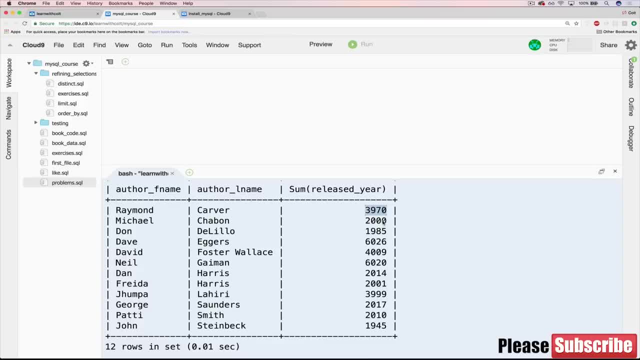 recently when I was compiling my taxes. Probably going to bore you to death with this, but I have a whole. I have a database that has sales data for every week for one of my projects that I have going on And I just wanted to figure out exactly in a given year, how many sales or not. 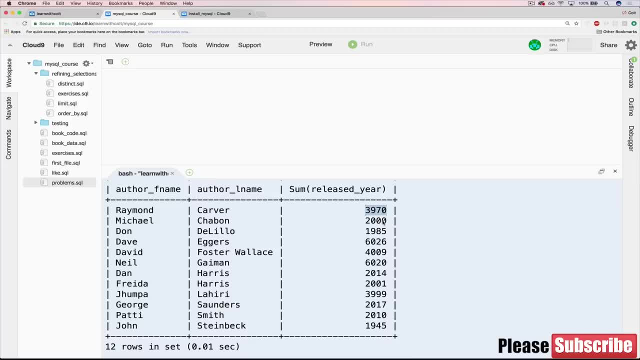 how many, but how many dollars I'd sold in that entire year and just add all those values together. I didn't want to, you know, manually enter them into a calculator, So it was just a matter of using select sum. And I actually did a select sum with a group by, because I grouped by year. 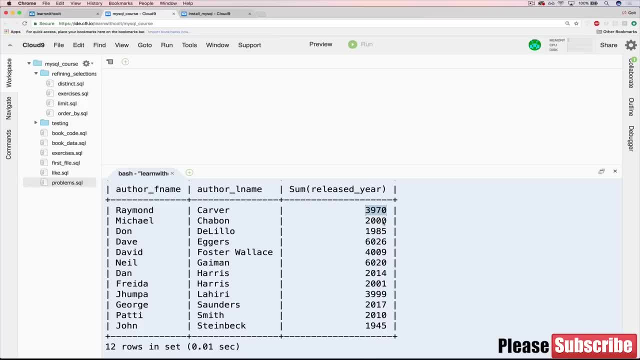 because I have sales going back I think 2016,, 15, and 14.. So I only wanted 2016 for my tax season. Anyways, if you're still there, thanks for making it through that. I know taxes are. 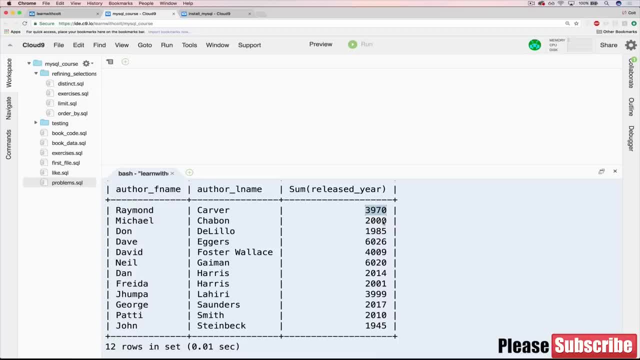 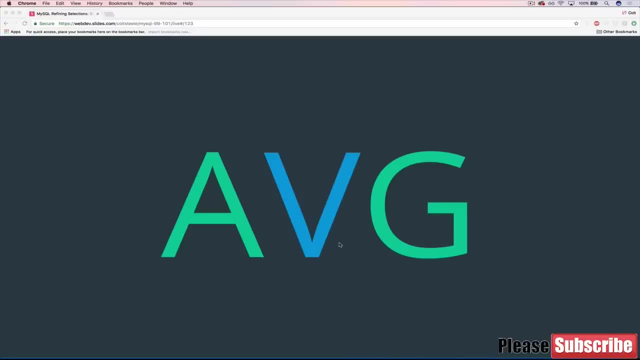 not the most interesting subject, but, yeah, some can be useful sometimes. Oh boy, I'm going to end it now. That was just bad. Next up, we're talking about AVG- Hang on. Next up, we're talking about average And, as you might have guessed, because I've said this for pretty much every video in 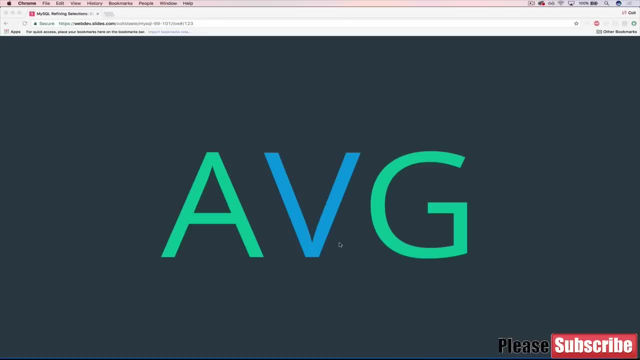 this section. it does what it sounds like. Actually, that's a lie, It sounds like AVG, but what it does is average data, So it will sum things together and then divide them based off of how many things are added together. So it's pretty useful if you're. 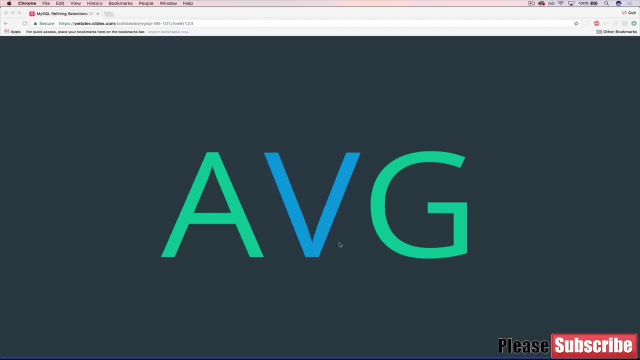 trying to do things like find the- I don't know- average sales for something in a given month, or find the average price of something in a database, or the average- I don't know anything- average number of users. that are the average number of followers that your YouTube videos have. 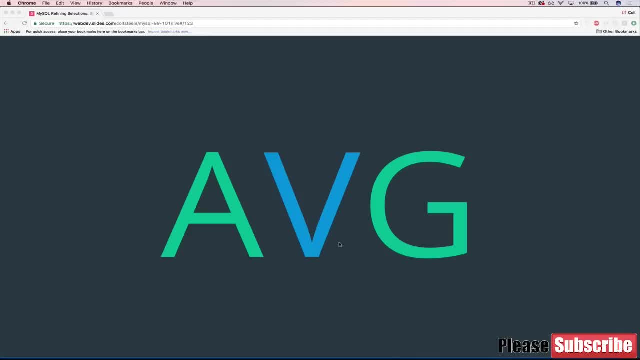 I mean averages are pretty useful In general. think of all the times in your life, Hopefully. I mean, I don't know, maybe you don't, maybe you never average things, but I feel like it's something I find myself doing. 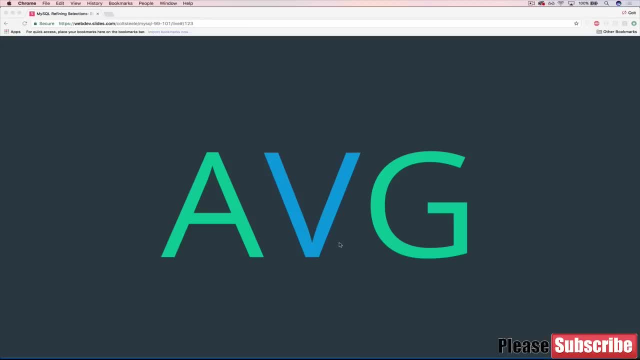 It's a lot of. what teachers do is find averages, average scores, average grades, Okay. well, let's just get back to this. There are a lot of uses for averages. It's not a perfect way of getting insight. I don't want to say that. you know, the average is this amazing. 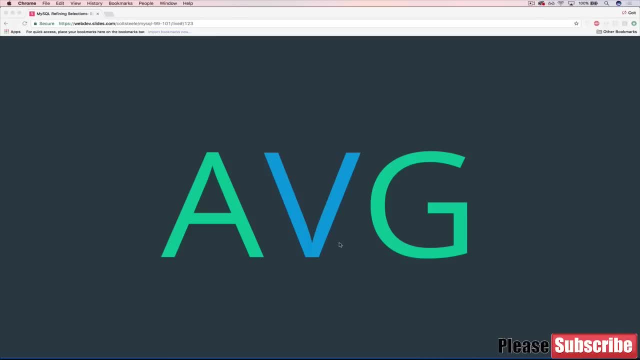 all-encompassing piece of data, but it can be useful, Anyways. so how do we use it? Also, as you might have guessed, I'm going to show you how to use it on its own first, and then how to use it with GroupBy. By now, we'll be able to do this pretty quickly. 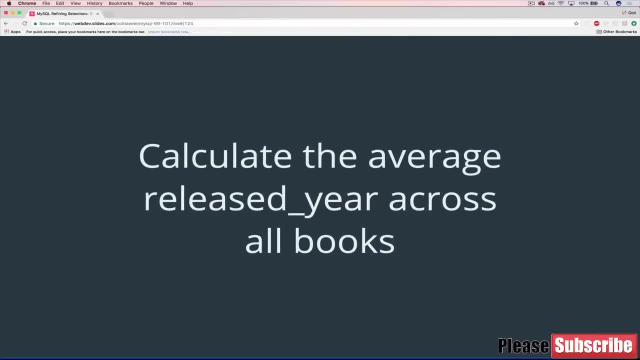 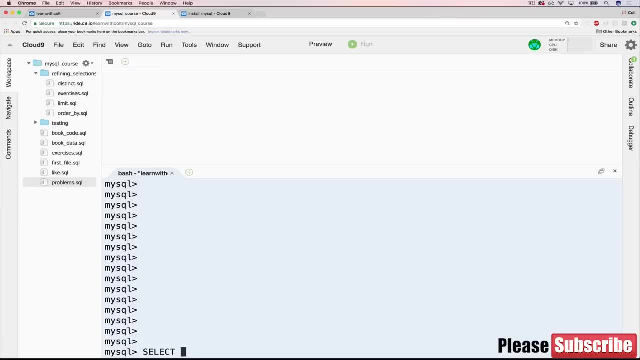 and it should serve as review. So we could do something like this: Calculate the average released year across all books, And that's very simple. We do a select AVG average released year from books And, as you can see, we get 1999.7895.. 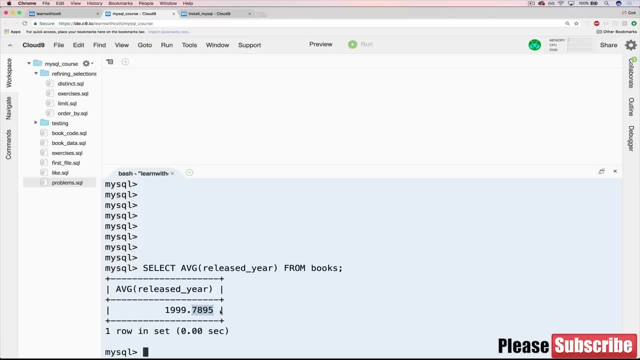 And it's important to note. yes, there's a decimal and it goes out to four places. here We'll talk more about different types of data- data types- in a coming section, where we'll talk about the differences between integers and the ways of storing decimals. But 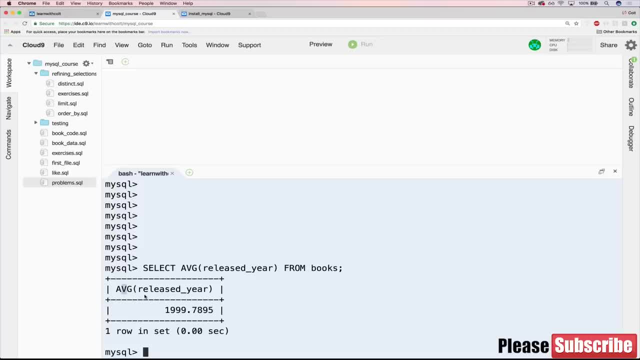 for now. it's important that you notice when you do average, it doesn't round things up to a whole number. It gives you four decimal points. We could also do things like select the average page count from all of our books, which is: 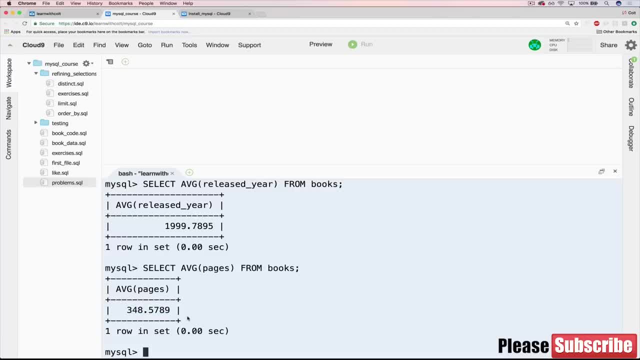 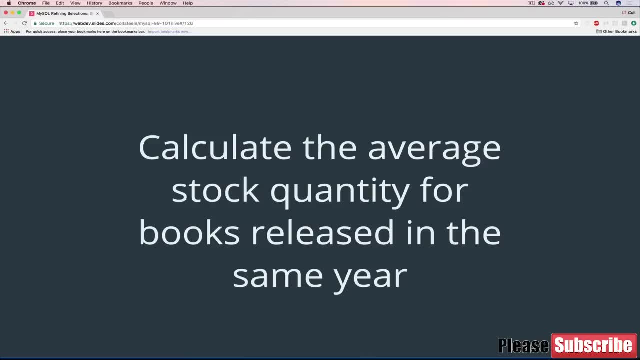 348.5789 pages. Okay, so now let's see how to use it with GroupBy. That's a more common application. How do we do something like calculate the average stock quantity for books released in the same year? So this is a little bit different. We're not grouping by author. In this case, we have a. 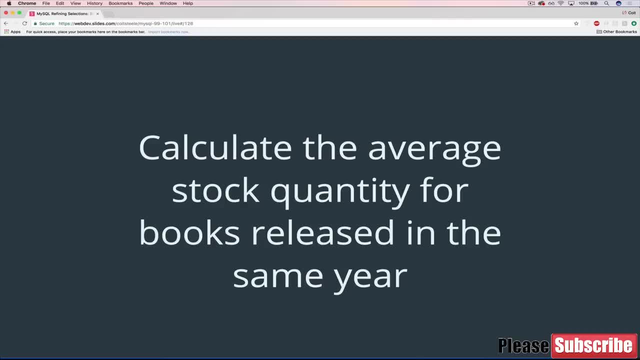 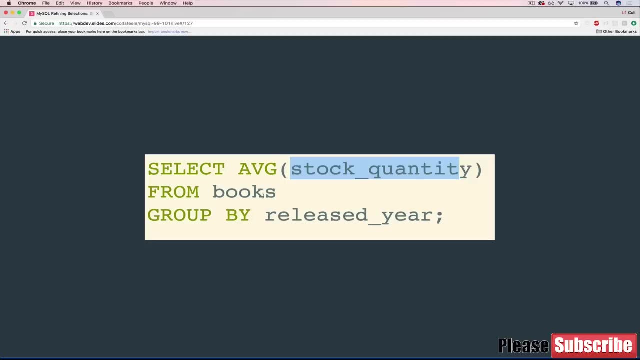 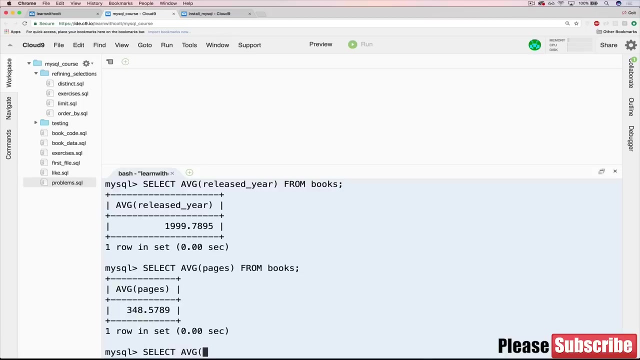 couple of books that were released in the same year by different authors And this is sort of arbitrary, very arbitrary. But how do we calculate the average stock quantity for books released in the same year? Looks like this: Select AVG- average stock quantity from books GroupBy released year. So let's try it: Select average And we want stock. 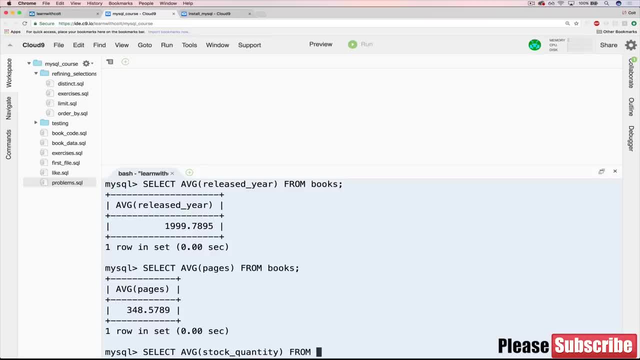 quantity: quantity from books GroupBy released year. Just like that. Not that insightful to look at, let's be honest. but maybe we could do something like this: let's print out the release year, the count, how many books were released that year, and then the average year. so it will look like: 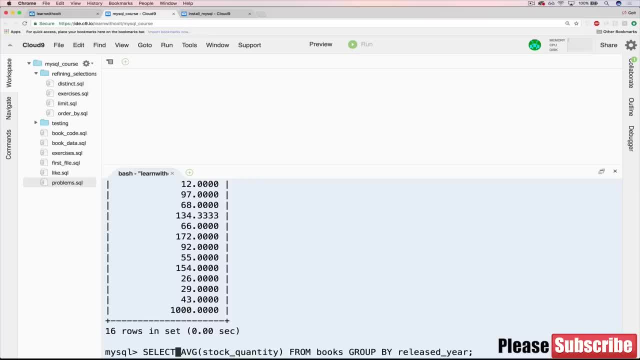 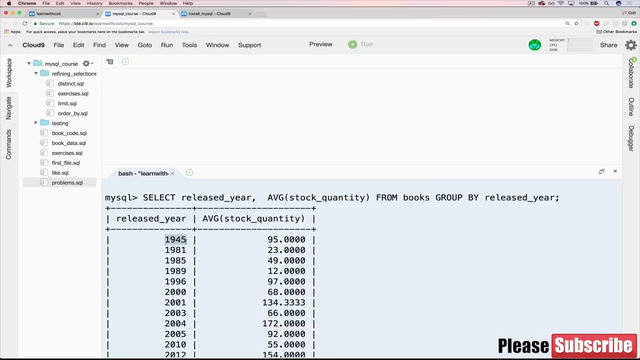 the average stock quantity, excuse me, so we'll have released year, and then let's also- well, let's just leave it at that released year and the average stock quantity, and if i do that, you can see: 1945: 95 is our average quantity. 2001: 134 is our average quantity. 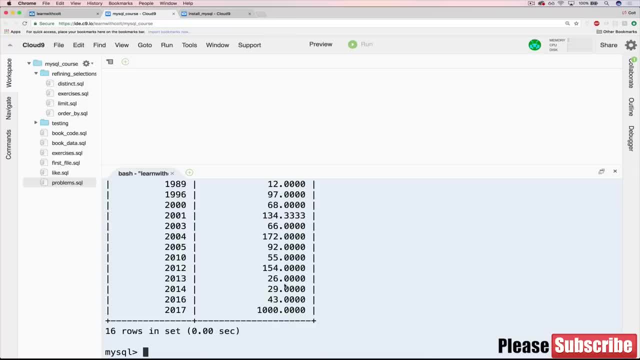 yes, not that useful, i totally agree. but i just want to mix it up because we've been doing a lot of group by author l name, comma, author f name and it gets kind of old so we can group by other important pieces of data. but of course we could do something like this: select: 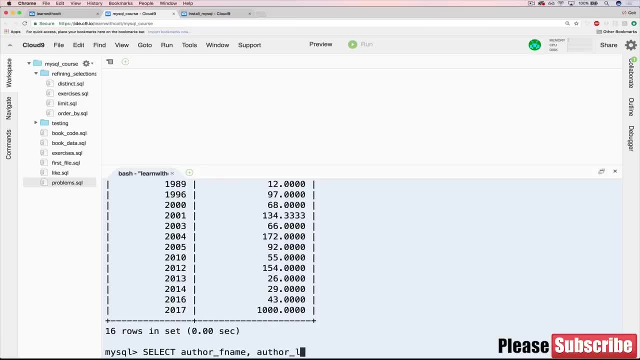 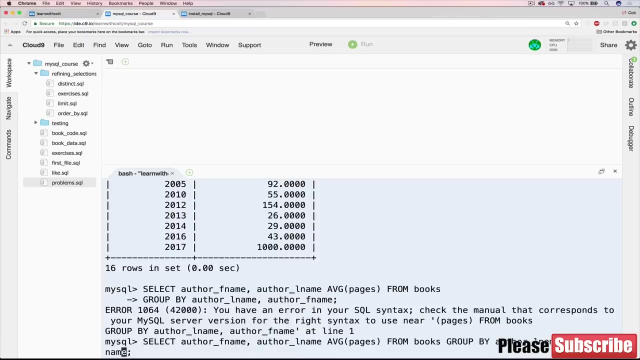 let's do our good old author f name, author l name and average. let's do average pages written by every author or each author from books group, by author l name. author f name. oh boy, it's a little bit too eager there. what's our problem? looks like i'm missing a comma. 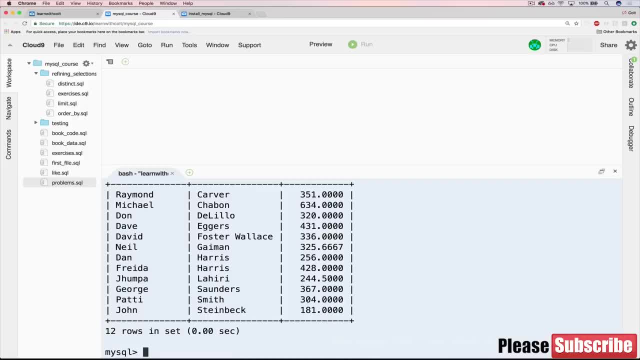 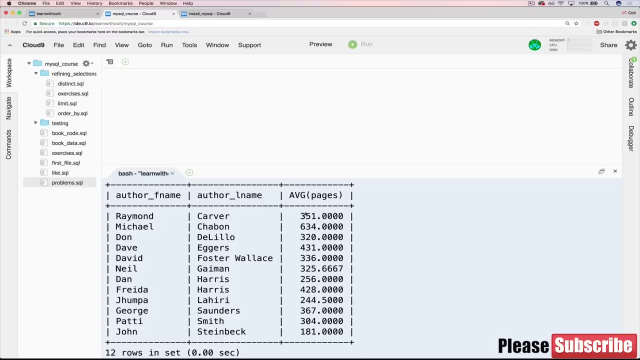 all right here. okay, so you can see the average pages written. we saw how to select the min and the max as well as the sum. now we have average. also, it's important to note that someone like, let's see, john steinbeck, who we know has one book, 181- it still adds the four decimal points. that has to do with 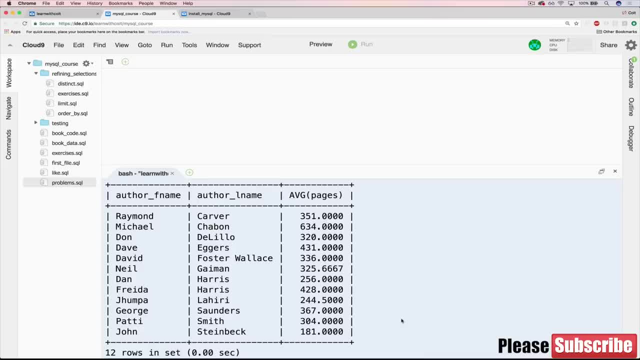 the data type, that this is um, and basically i'm just going to pump that one until we talk about data types. but i just wanted to highlight it here. you still get those four decimal points, even if it's an even integer, even not meaning- okay, that's a bad choice of words- not as in even. 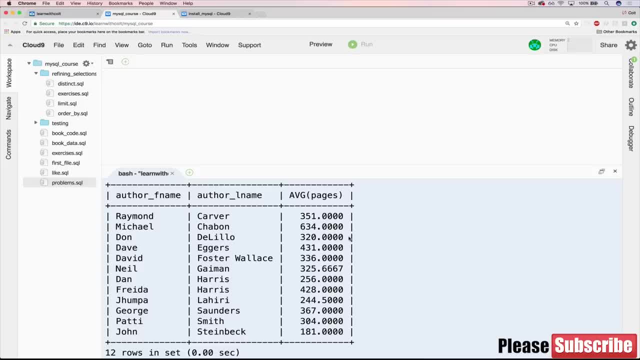 and odd, let's say as a whole number. there we go all right, so that's average and that actually wraps up the section on, or the new content on, these aggregate functions. so we saw count, well, we saw group by and then count min, max, sum and average, all different things that we can do. 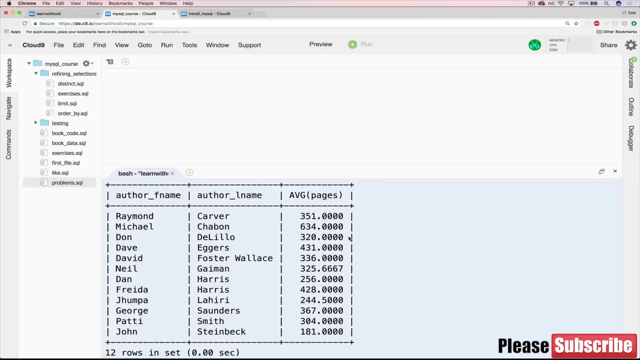 on their own or in conjunction with group, by all right. so now we're going to get another chance to practice it. hopefully you're looking forward to that and if you're not, it's still good to do. it's like you know vegetables, just got to eat them. i hope i don't offend anyone if you're a vegetarian. 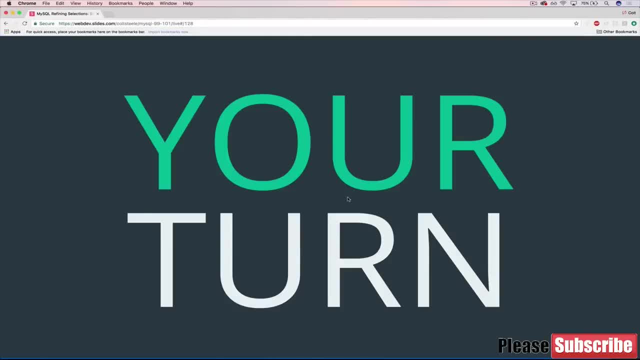 all right, all right, welcome back. it's me my cat. can you purr say? hi, that was my cat, i promise so in this video. we're now going to spend some time- or you're going to spend some time- getting some practice with the different functions. we just saw things like count, min, max, sum and average, as well as using them with group. 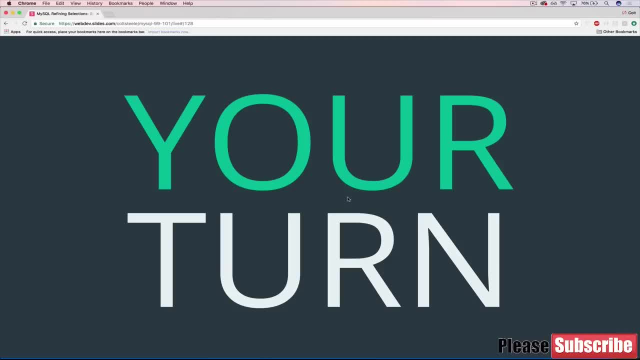 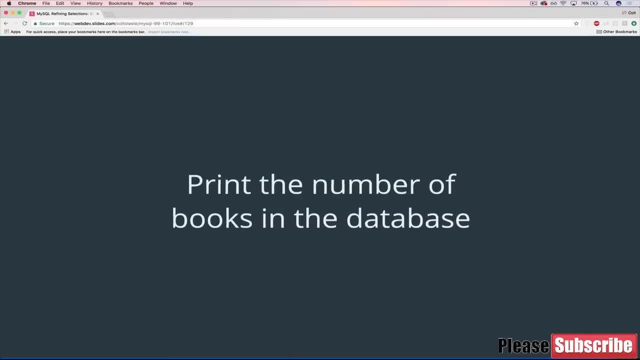 by. so in this video i'm just going to lay out the challenges for the exercises and then in the next video we'll talk about solutions. so the first one is to print the number of books in the database. so you know, don't just do a select star from books and then manually print. 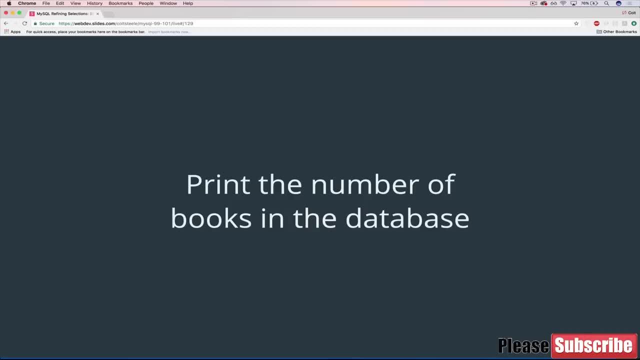 go through and tabulate or count them, write a single line that will print out the number of books in the database and then, once you've done that, move on to this one. print out how many books were released in each year, and i have to say the wording on some of these is it's not great. 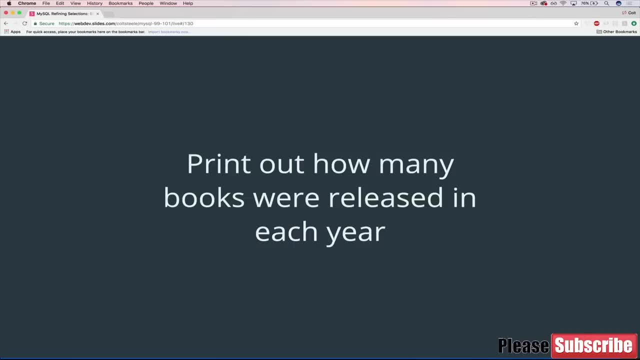 but i kind of struggle to figure out how to explain this. the best way basically group things by year that they're released and then just print out how many were released that year or each year. so it should look something like 2005, one, 2006, two books. 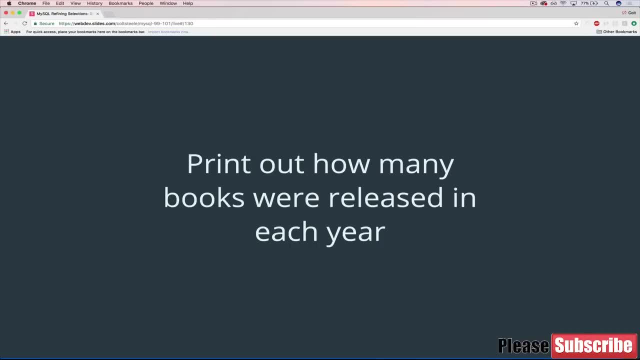 1945: one book. now, those numbers i just made up, so don't worry about those numbers. but basically that's the idea. you should have the year and then account for how many books were released that year and then next up print out the total number of books in stock. so there's a stock quantity. 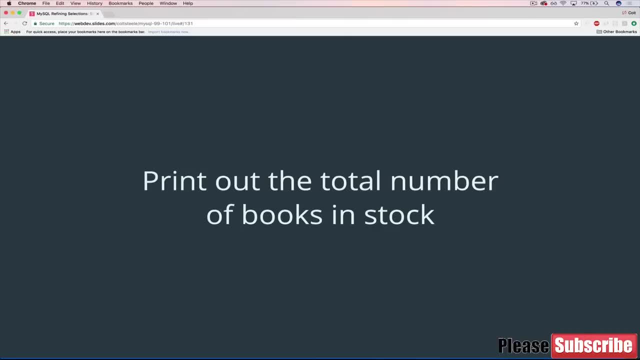 and every book has a stock quantity. so print out the sum. ah, i just gave it away. well, print out the sum of all of the books in stock. so just add together all the quantities and then find the average released year for each author. so you'll need to go through. 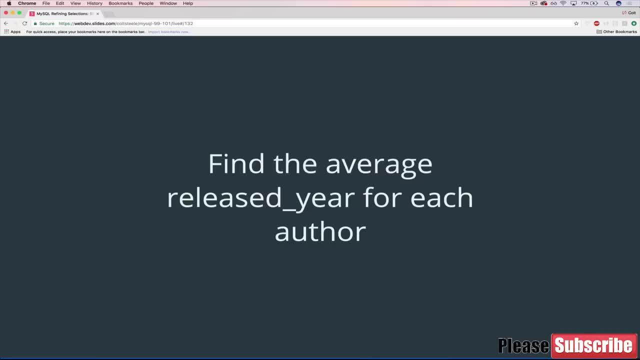 group things by author first or last and first name and then find the average year that they were released for each author. so your results should look something like raymond and then carver, and then the third column should be the average released year. let's say that's 1985.2 or something. 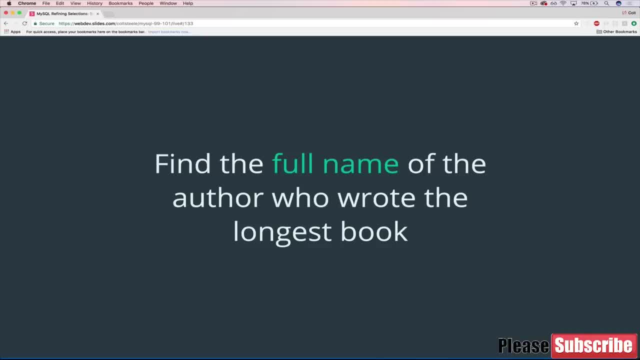 next up, find the full name of the author who wrote the longest book. so full name here is in a different color because it's a little different. um this one. you'll need to, uh, use one of the tricks that we saw in that description to by publishing August 1st or something like that. so that's the. 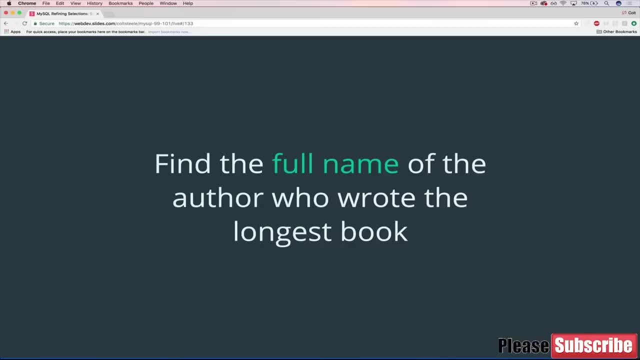 average release year for each author, and then we have a number which is the year that they were released for. so your results should look something like Raymond and then Carver, and then the third, that video where we talked about man and max and that issue. my cat's being a nightmare. hey, hey, come. 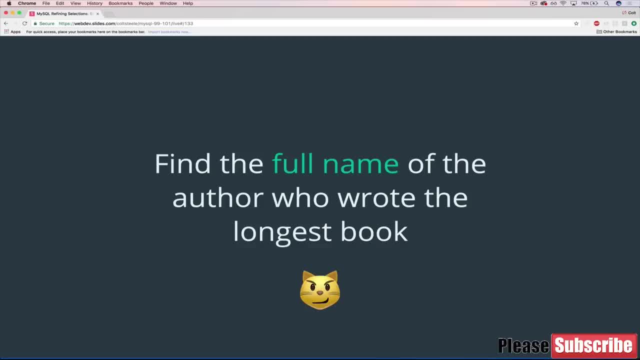 on hello. no, no, oh, my god, she's just knocking everything off my desk. hello, okay. so where was i? the idea here is to not just find the longest book or the page count for the longest book, but actually print out the name of the author, the full name. so you'll need to use concat. 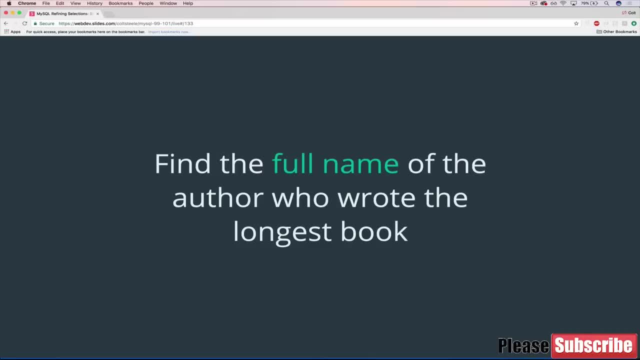 full name. we want first plus last name, with a space in between, of the author who wrote the longest book. so you need to find the longest book and then use that to find the author. basically, and there's a couple ways of doing that. if you remember the min and max video, that 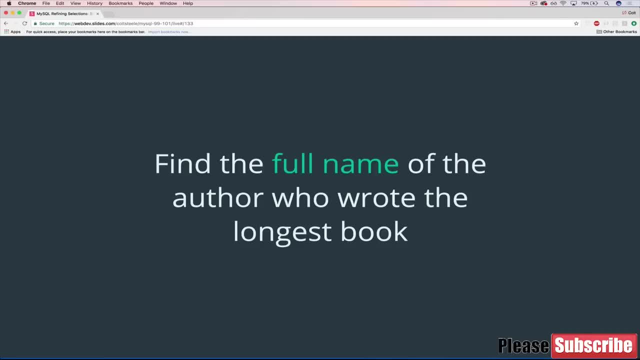 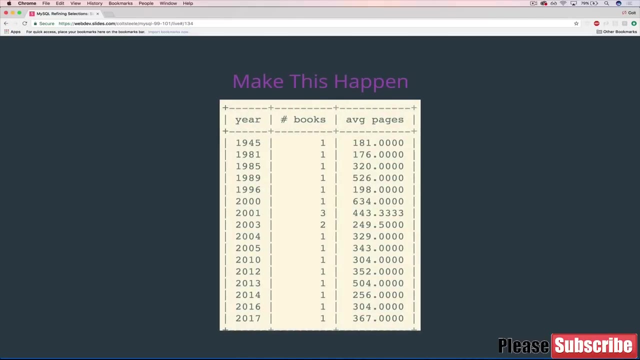 the second min and max video, where i talked about some of the problems, or one problem in particular, that arises when you try and print information like title or author based off of something being min or max, and then the last challenge here is to print this data out. so we should have the year is. 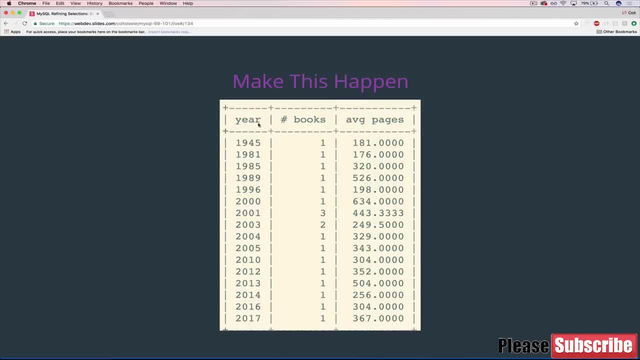 released. notice that we have an alias for all three of these. so the year like 1945, the number of books released in that year. so you know one, one, one one. but then here we go in 2001 there average number of pages for those books released in that year. so i won't tell you how you need to. 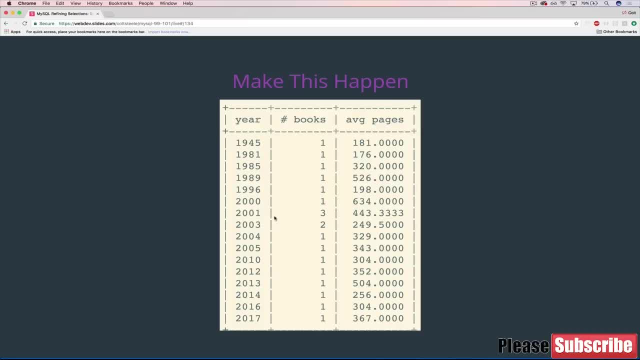 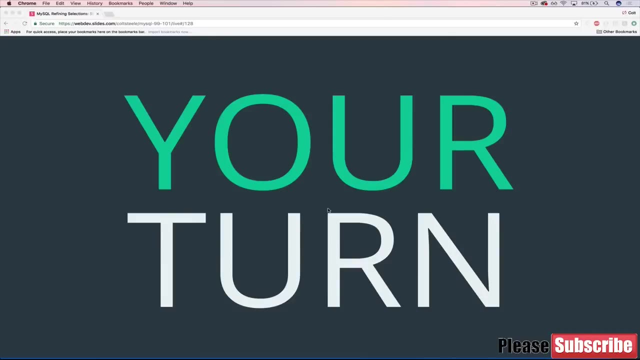 group things in this case, but hopefully you can figure that out based off of this image. all right, i gotta take care of this cat situation. oh my god, and then in the next video we'll have a solution. okay, so in this video we're just going to go over the solutions to the exercises i 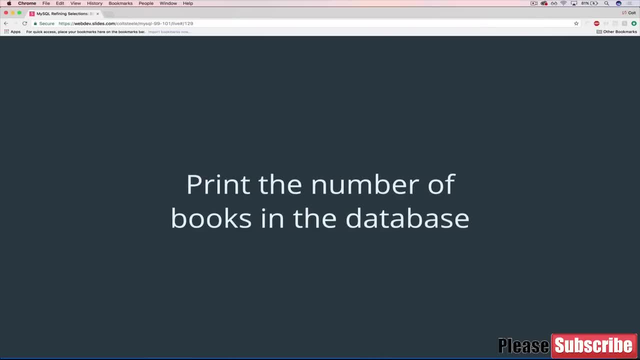 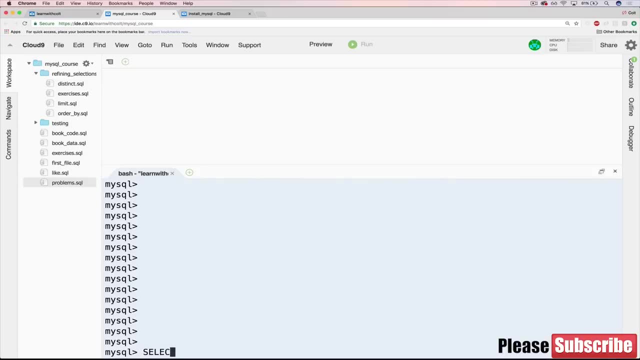 introduced in the previous video and the first one here is to print the total number of books in the database. so we'll need to use count and all that we'll do is write a select count star from books, just like that, and we get 19.. all right, and that's it. 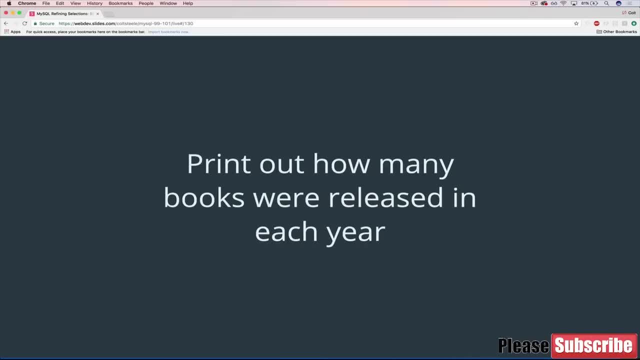 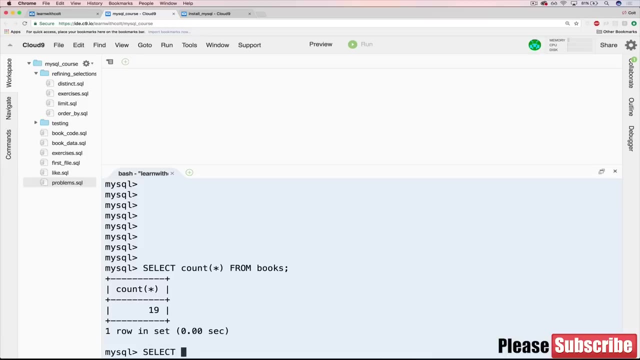 the next one is to print out how many books were released in each year. so we'll need to use a group by group by released year and then use count in conjunction with that. so let's do a select and we'll just do count star from books group by released year, just like that. 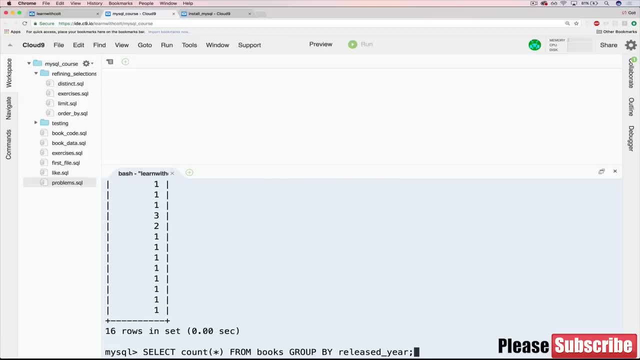 now. on its own this isn't that useful, so i'll go ahead and add in select released year comma count so that we get the total number of books that were released in each year. the year is released and then the count you can see. most years have one book released. 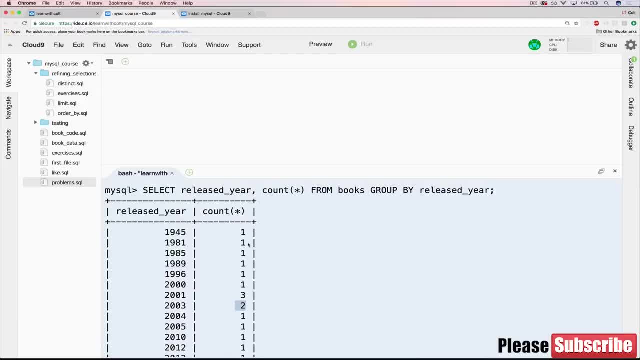 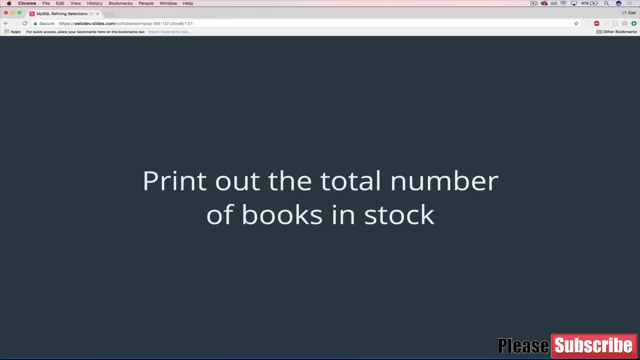 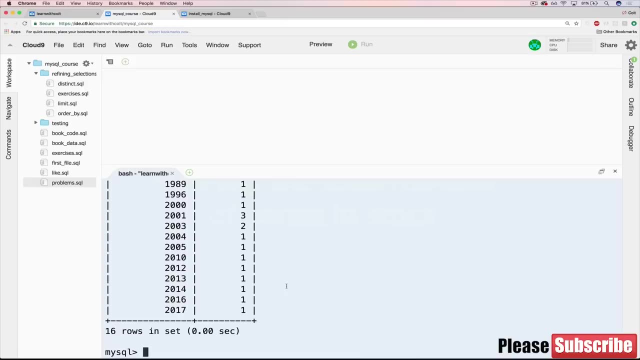 2001 has three. 2003 has two. all right, so the next problem: print out the total number of books in stock. so this one you'll actually need to use sum. you'll need to sum all the stock quantities, which is something i guess we haven't really used. 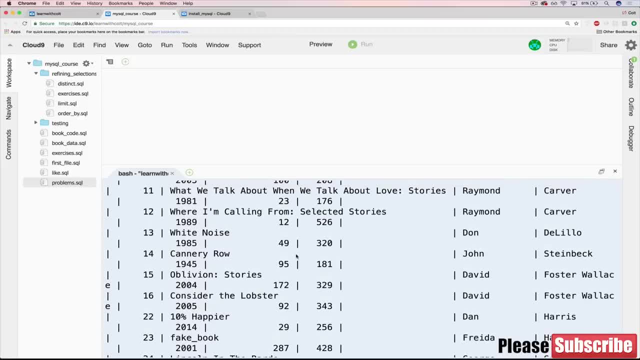 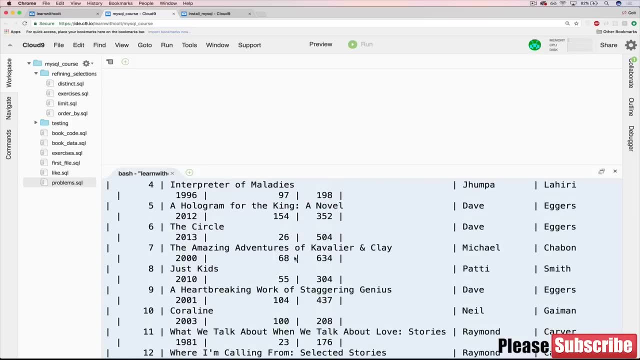 that's not how you spell from. we haven't used stock. oh, my cat, you gotta chill out blue. so stock quantity is not a piece of data that we've used very often, but it is here. we've neglected it a little bit, but it is there, as you can. 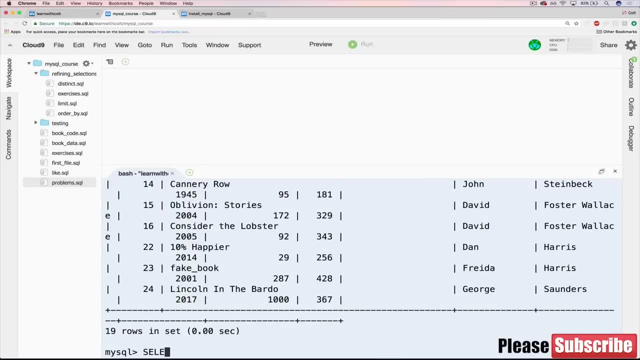 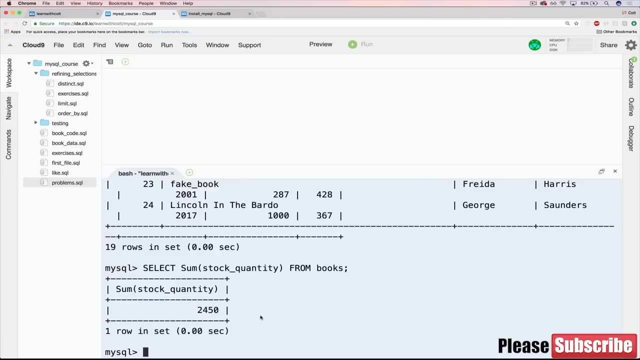 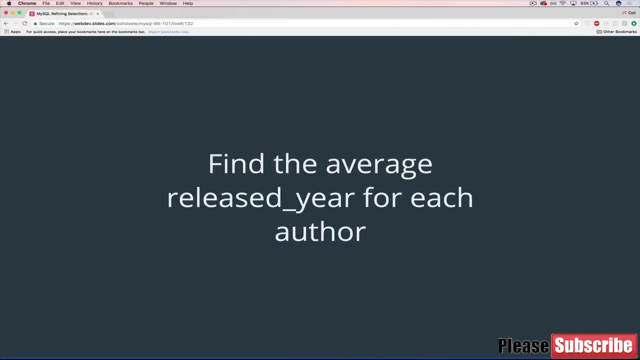 see. so we just want to add them all together and that's just going to be select sum, stock quantity, quantity, quantity from books. there we go. we have 2450 books in stock. so the next problem here is to find the average release year for each author. so we'll need to group by author and then we'll need to use average abg. 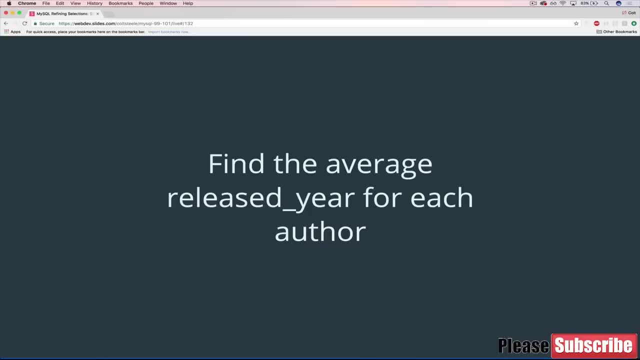 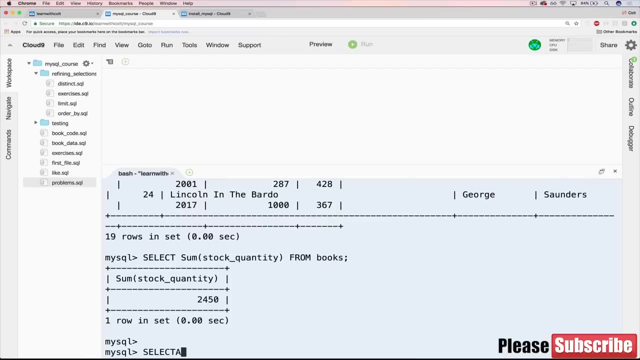 to calculate the average release year. so let's give it a shot. average release year for each author. so we'll need to do a select average and then release year from books grouped by. and then we're grouping by author, so we'll do l name, comma author, f name. 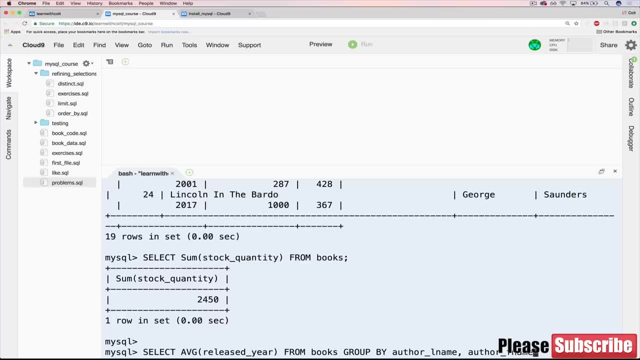 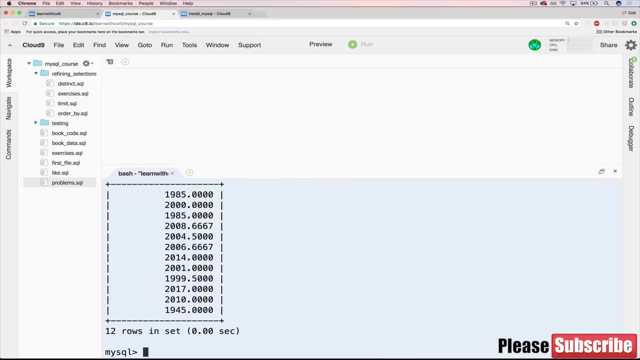 again because of the harris issue. uh, what are their names? dan harris and frida harris. okay, so if we do that, oh my god, my cat again. oh boy, well, i've taken care of that and i don't mean wow, apparently i have not taken care of it. 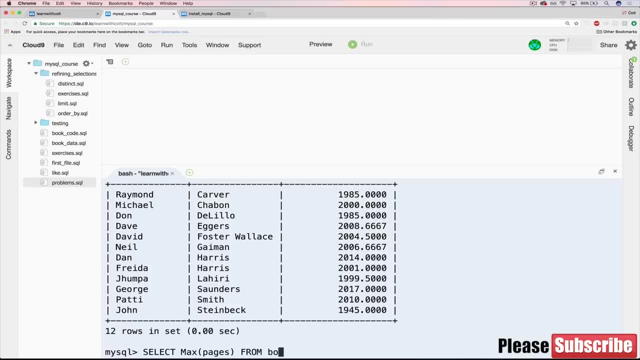 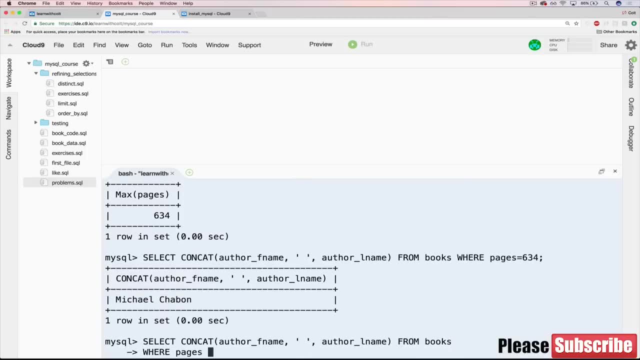 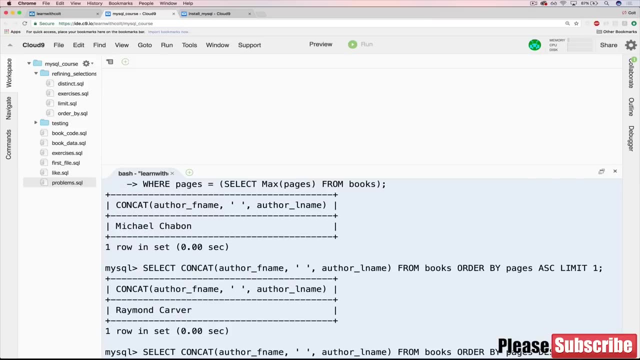 all right, hang on. so back to the problem at hand. this works, we're getting average years. but to make it a little bit better we should also add in the author f name, comma author l name, just so we can make a bit more sense of the data. so now we can see raymond carver's average release. 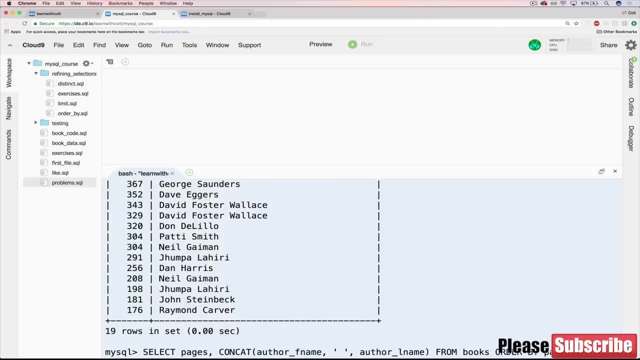 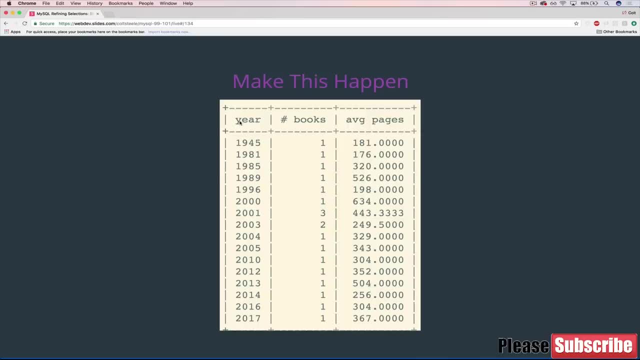 1985.. um, let's see. neil gaiman says 2006.6667. all right, so that's all there is to that problem. now we get to the one that's a little different. find the full name of the author who wrote. 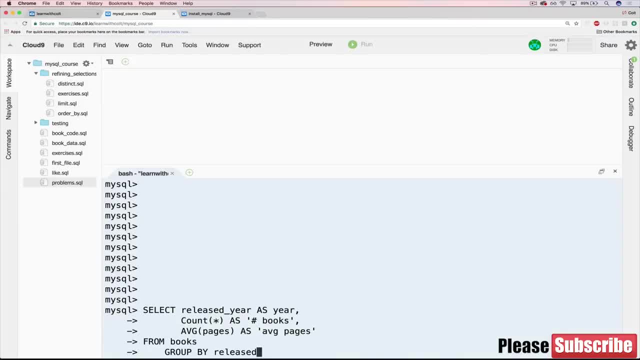 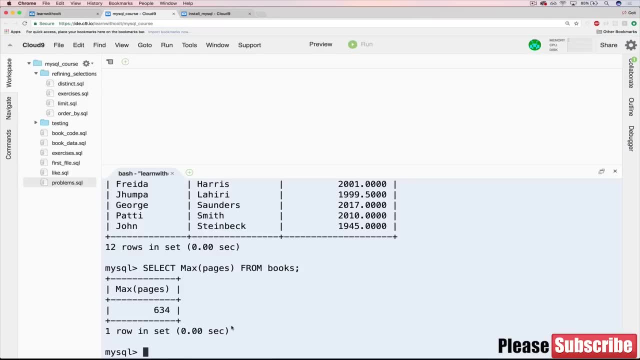 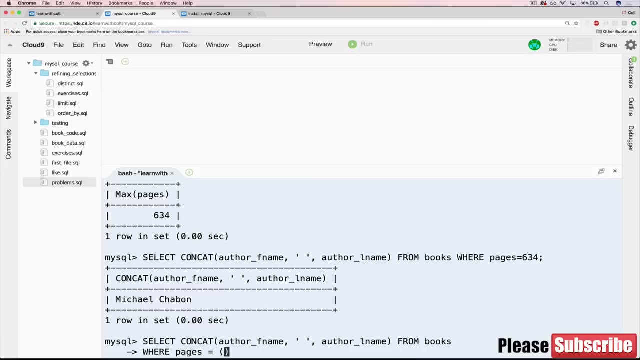 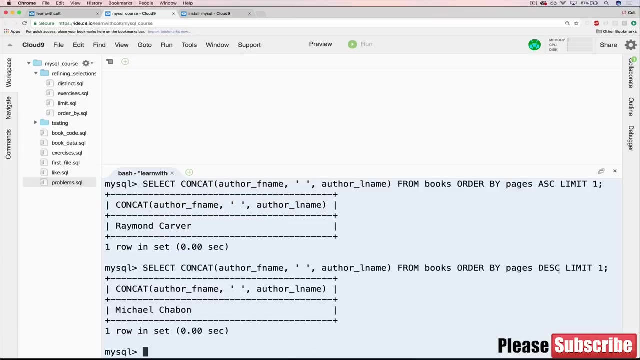 the longest book. so there's a couple ways of doing it. the the way that doesn't qualify as a solution. the two-step process would be first to find the longest book, so that would be select max pages from books like this 634, and then, you know, at this point we can make a second query. 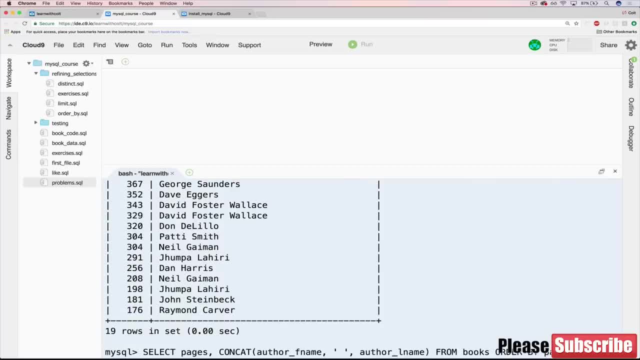 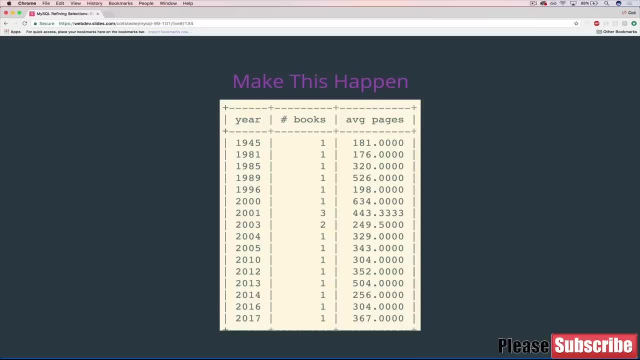 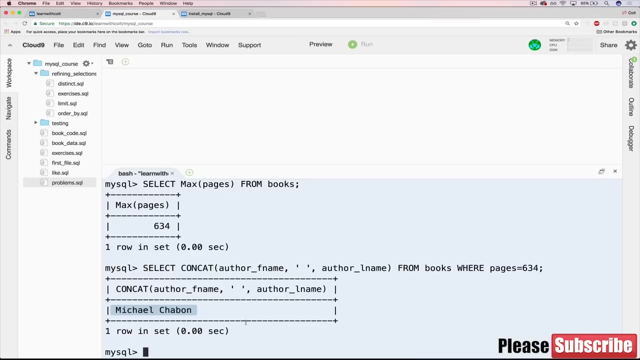 select and we want to concatenate first name and last name, so we do concat: author f name, comma, author l name and we want to space in between, like that from books where pages equals 634, and there we go, we get michael chavon. however, we want to do it in. 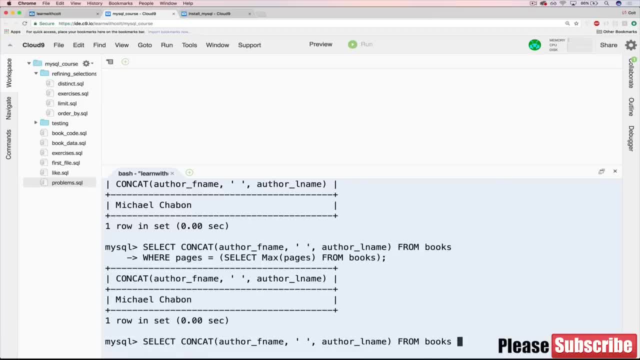 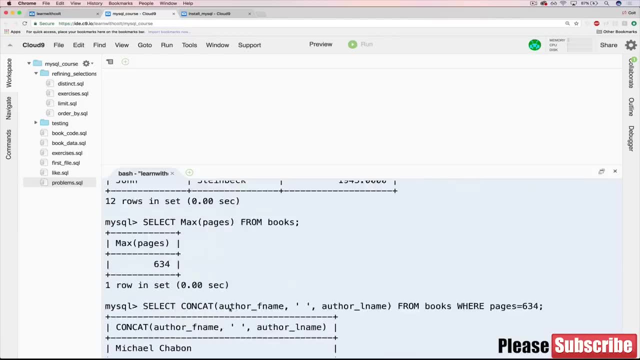 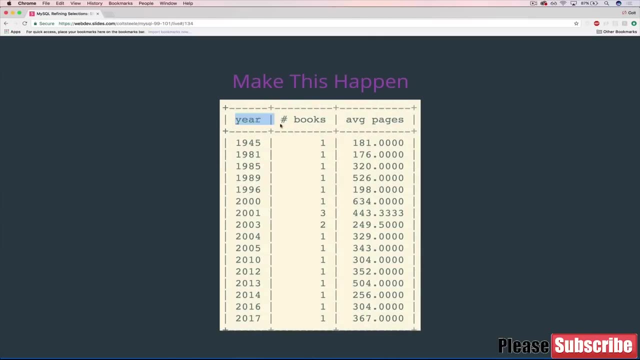 one step. so we can either do the sub query route, so we'll do select concat author. however, instead of uh, we'll do from books. but instead of just doing where pages is 634, we'll do where pages equals, and then we use parentheses for the sub query. hopefully you remember this part. and then 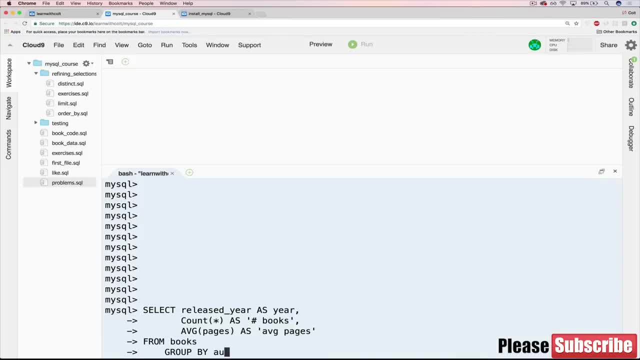 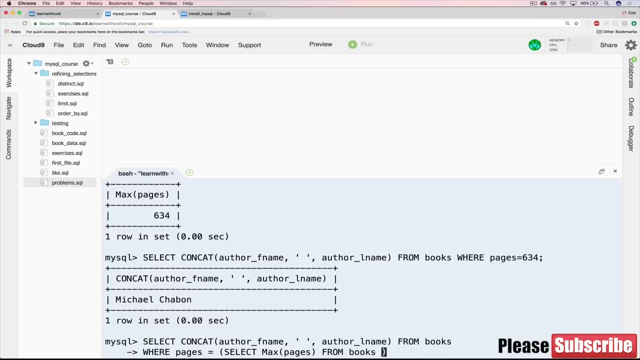 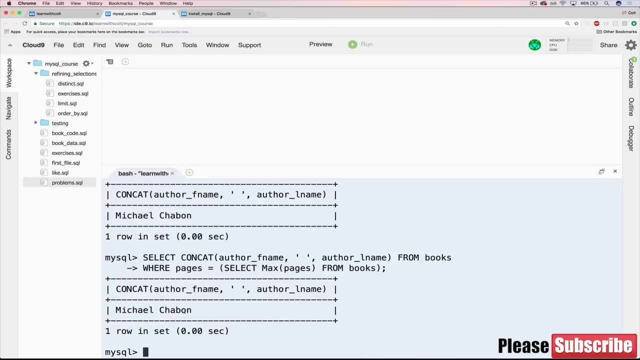 in here. all that we do is write our query, so that's going to be select max pages from books, and we get the same thing, michael chabon. and then there's the other way of going about it, which is to not use max at all and circumvent that, which is actually fast. 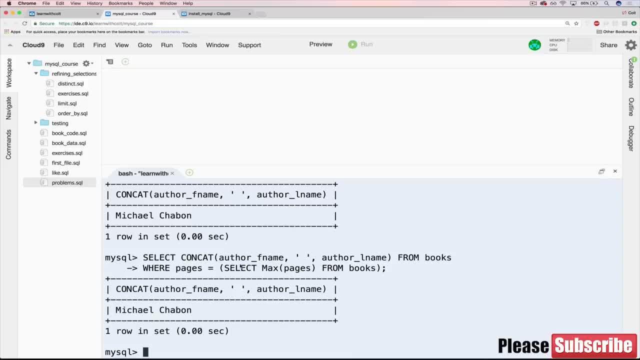 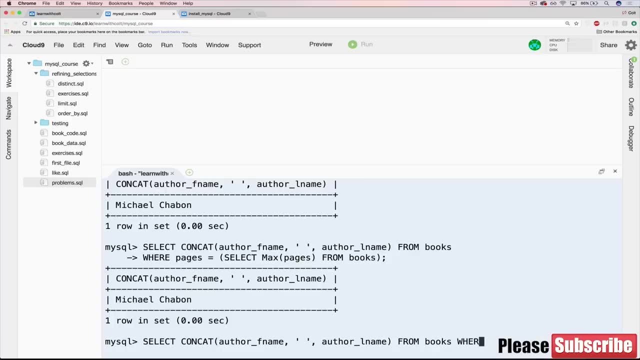 so that'sチーム of order means you're going to do it faster, to use order by and then limit it to one so we can do the same thing. so, like in cat: author f name, author l name from books and then we just do an order by pages ascending limit1. 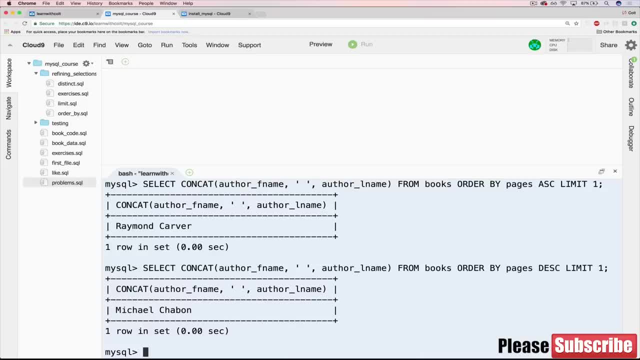 and i believe i have that backwards. we want the longest book, not the shortest one. there we go on it in descending order so that we get the longest one at the beginning and that's going to be 634. so if we, you know, if we get rid of this limit one and actually if we get rid of the limit, 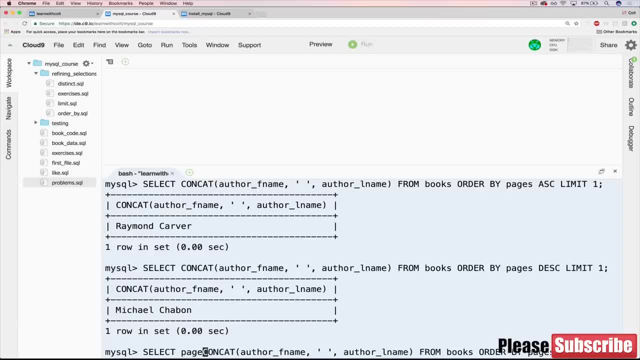 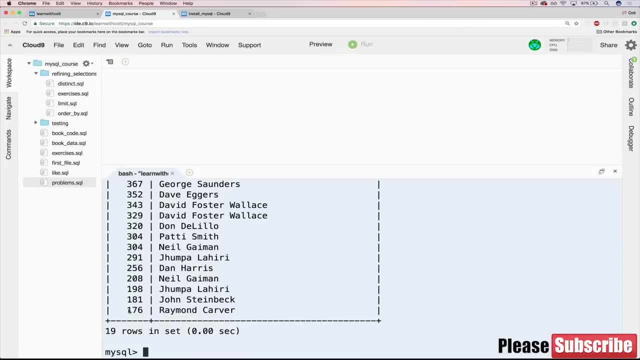 one and let's do pages comma. all right, so you can see, now we've got 634 all the way down to 176, and i was. i had it backwards. um, okay, so both are valid ways of getting a solution. this one is a little bit uh. well, it's a little faster because we're running one query. this version, uh, is more. 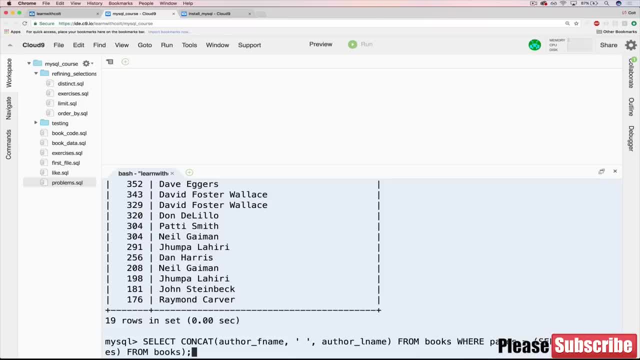 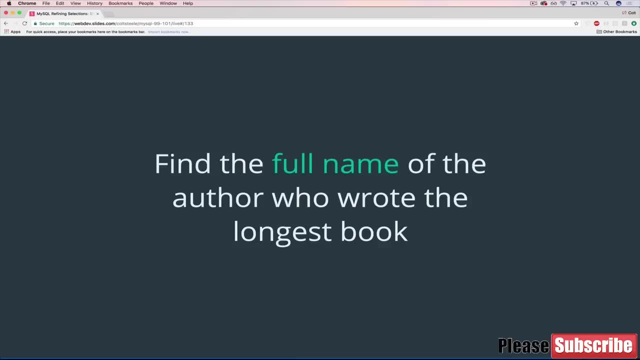 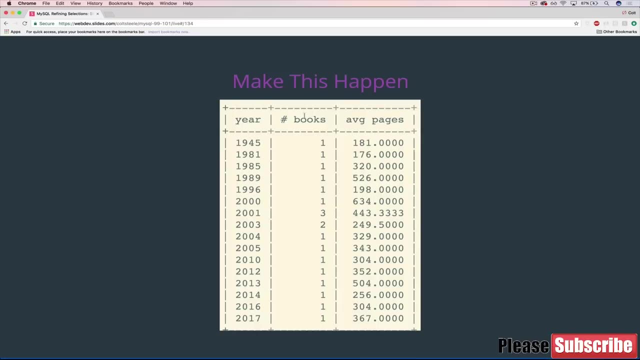 complex, more advanced, i guess. uh, but i would definitely stick to using this when possible using order by all. right, let's move on to our final challenge here. make this happen, make this happen. so we've got a couple things going on. we've got a year, so things. let's see, we've got a year. 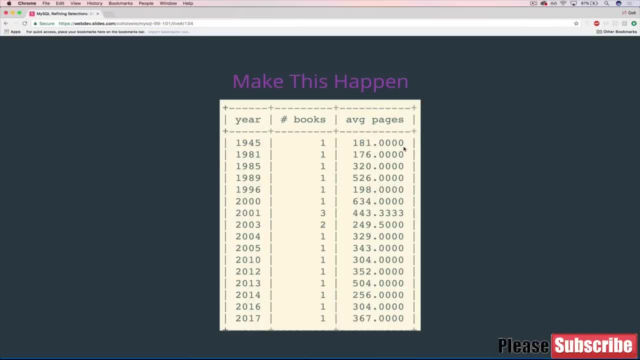 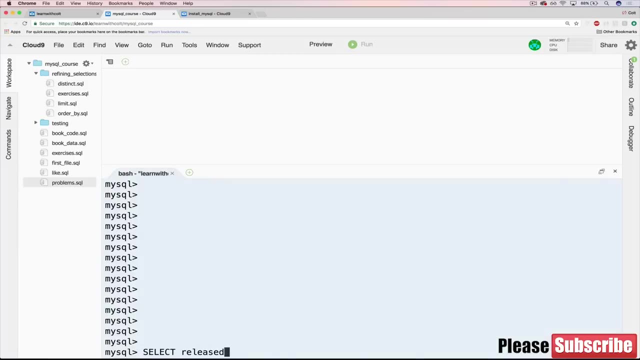 the number of books in that given year and the average pages for all those books for that given year. so things are grouped by year and we have three aliases going on. okay, so let's give it a shot. so we'll start off by selecting year or released year and giving it the alias of year. 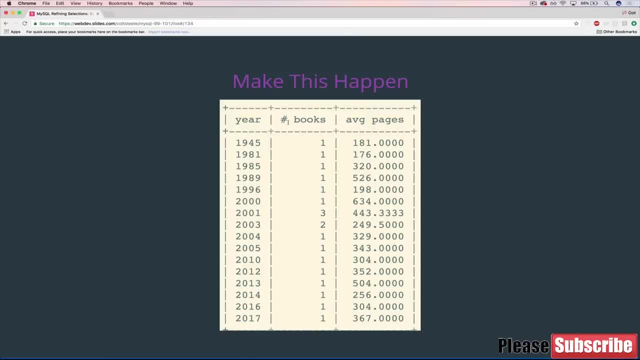 then the next thing is the count. remember we're going to have a group by at the end. so we're doing all of this, you know, writing the three things we're selecting before we actually have the group by, but at the end we're going to have group by released year. so this here, number 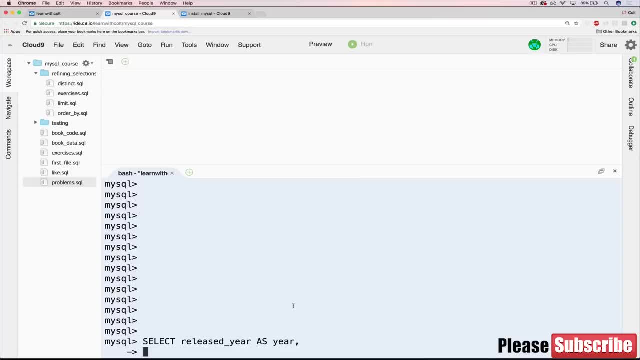 of books is count. it's a count of the number of books released that year. so i'll indent and just do count. star as- and i need quotes here because we have that, uh, octahedron and i need quotes here- the thorpe, i think, is what that's called, the hash symbol as well as a space, so we need quotes for. 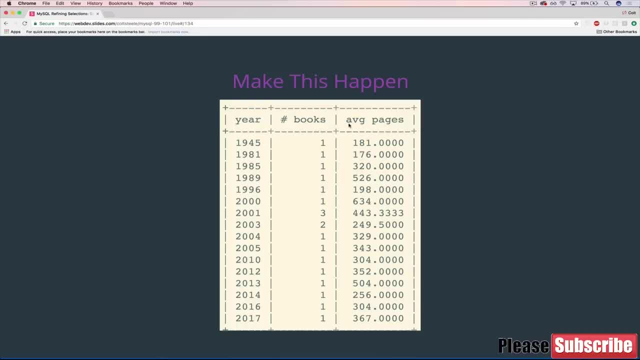 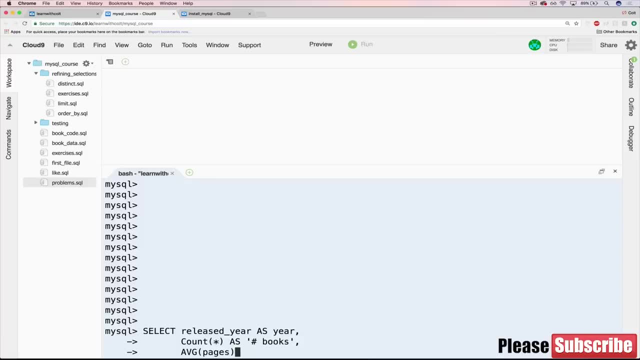 our alias. if we want to match this, then we have average pages. so it's going to be the same thing as far as our alias is concerned. so we need average number of pages as avg pages. is that correct? there we go okay from books, and you know i'll indent this one too. 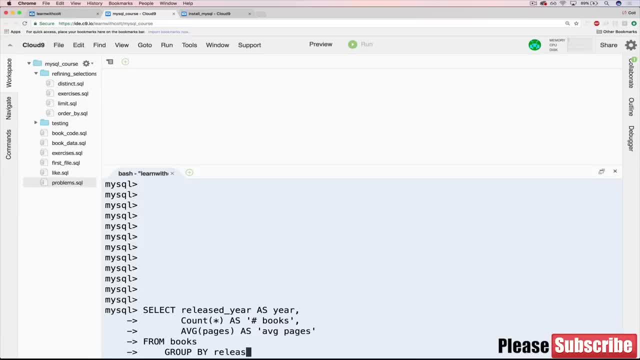 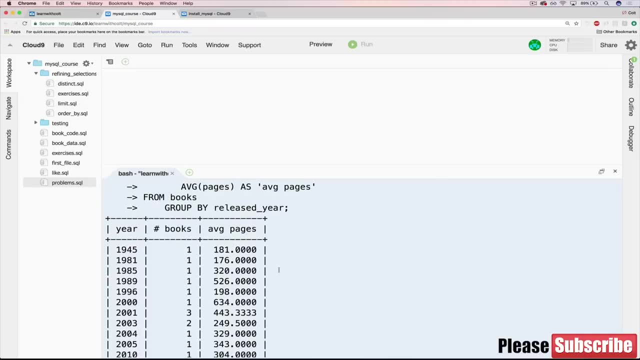 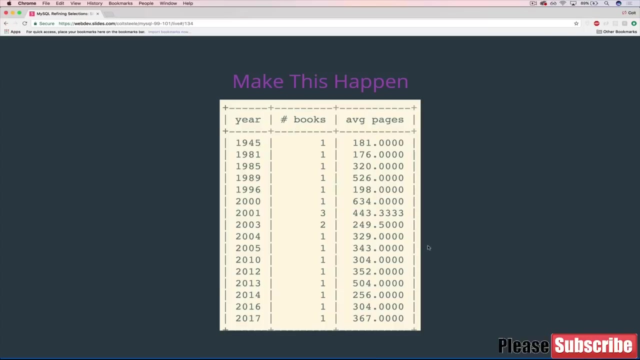 and we want to group by and we want to group by released year, hit, enter and pray and it looks like it worked out. 1945 had one book, 181 pages long. take a look at like 2001, there was three books and the average number of pages is 443 and a third. all right, so that. 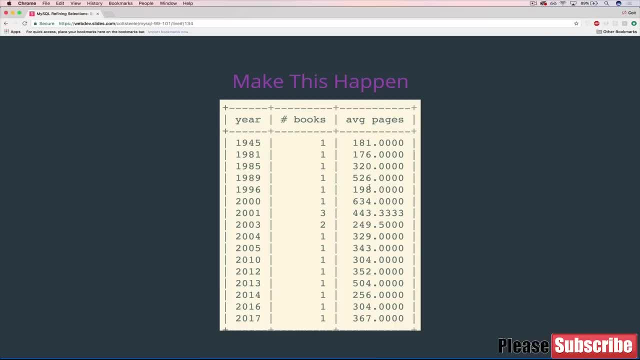 matches what i had here, which means that we got it right. don't ask me to do it again. i'm not going to do it again. don't ask me to do it again. i'm not going to do it again. i'm not going to do it again. 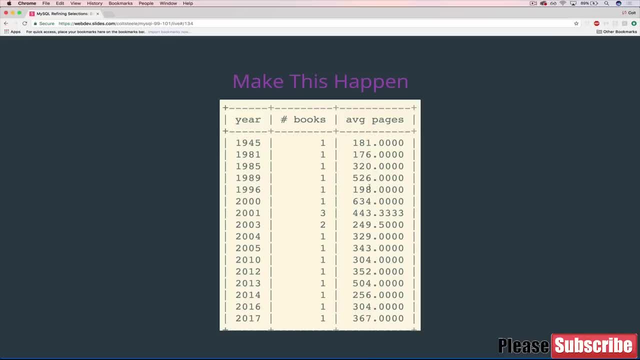 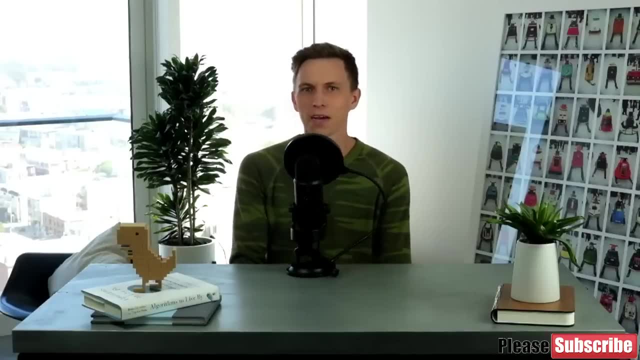 why you would do this. just don't ask. that's it for this section, and uh, yeah, i'll see in the next section. hello again, welcome to the next section. so first of all, hopefully you can see me- i am wearing camouflage. i know that can make it a little challenging, but i am here not just a. 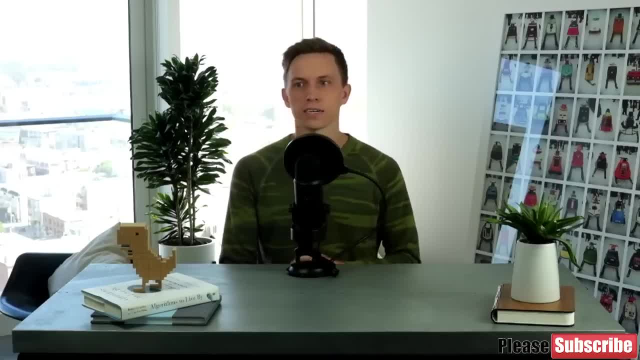 floating head. um, with that said, this section is a- well, i keep saying important, everything's important, but this section is really taking us back to basics. uh, in a way, we're talking about data types. so, if you remember, way back, i don't know- section three ish, i mentioned that we would 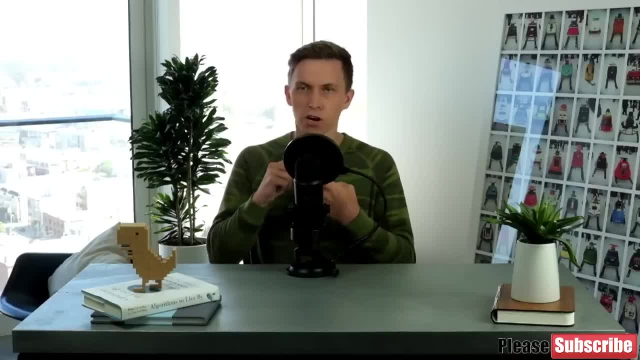 come back to data types. when i introduced varchar of our car, however you want to say it- um and integers are two data types we've been working with which are great, they're very useful, but there's a big world outside of those. what about things like, uh, decimals? how do we store currency? 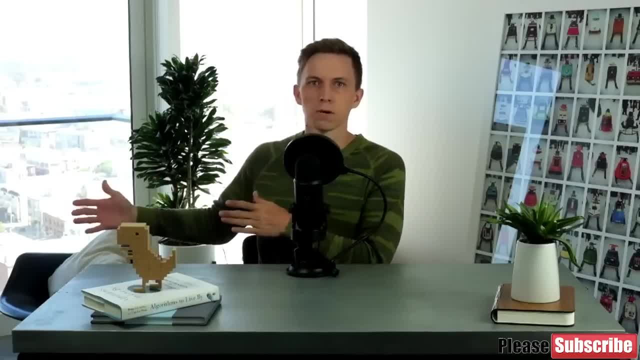 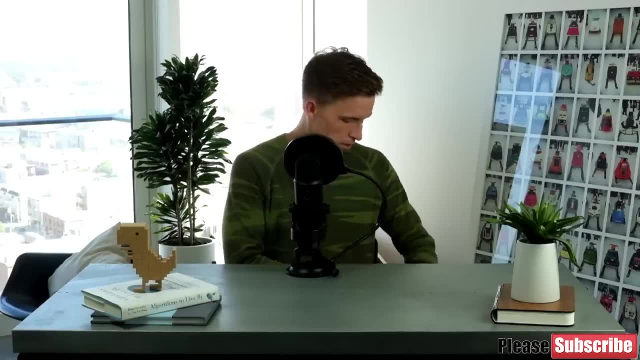 you know price information, where we have information after the decimal. how do we store things like, uh, dates and time? well wait, where'd my watch go? uh, things like dates and times. there's a lot of information that we need to store that doesn't neatly fit into varchar or integers, so this section is all about. 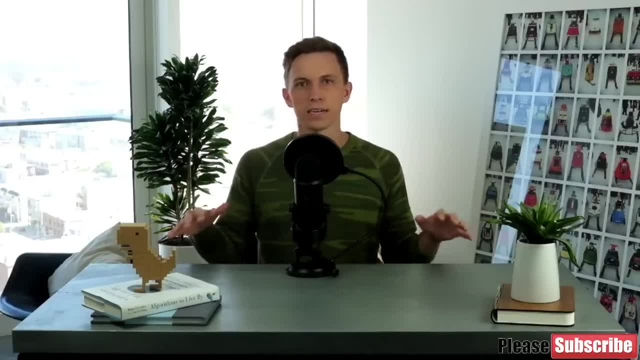 introducing and surveying those kind of different data types, and i could have done this early on in the course, but i've done it in the past, like that in person, and i find that students get too bogged down just worrying about all the data types when really they need to be focusing on things like 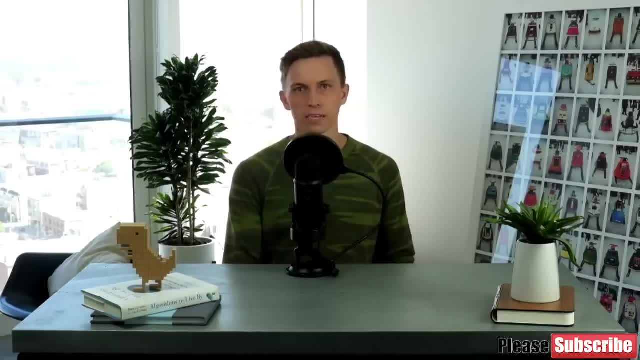 equals and insert statements. you know that's the focus of sql and mysql. we can insert, we can add new data types easily. so that's what this section is. we have the two we've been working with. now we're adding a bunch more, a ton of exercises here. nothing, you know, complex with our data. we're not, you know. 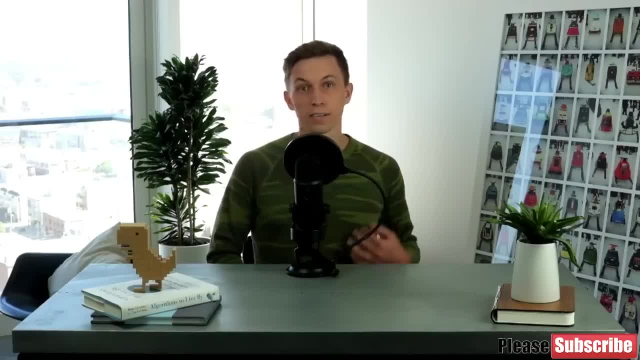 using any brand new data set. all we're going to focus on are the data types we'll see. in particular, we'll focus on dates, times, date times, time stamps, all this terminology- it gets a little crazy, but we're going to simplify that in this section. all right, see you in the next video. okay, so we're. 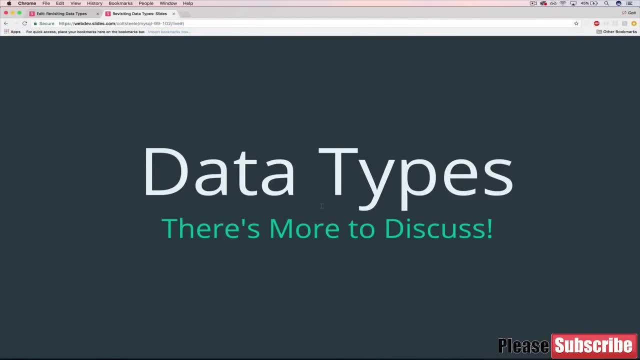 moving on now and it's time for a brand new section. in this case, we're spending some time revisiting something we've already discussed, which is data types. so very early on one of the first videos, once we got everything set up and installed, one of the first videos was on very basic data. 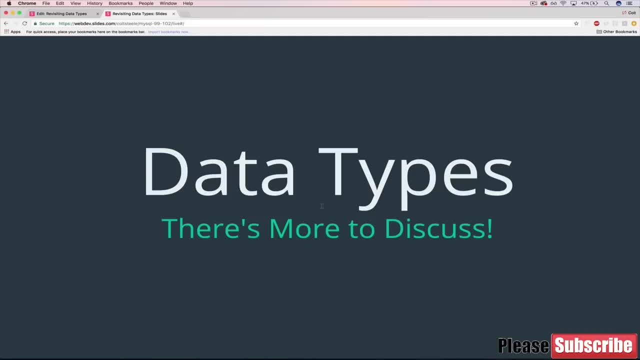 types. we talked about how data takes different forms and you have text and numbers and i kind of left it at that. we talked about varchar and int, our two first data types, but i showed you that there are a bunch more. well, now it's a time that i promised we'd revisit, we'd return to those data. 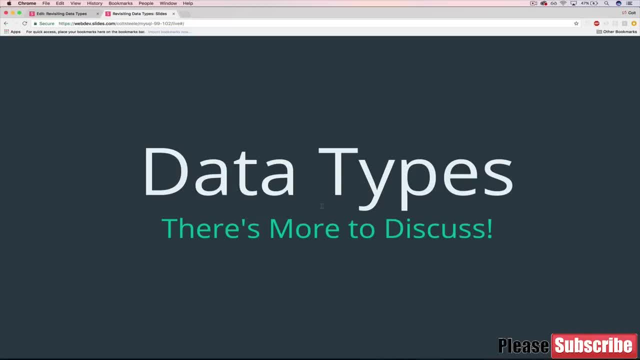 types and go into a bit more detail in depth around the some of the important data types. so we're still not going to go over every single one because a lot of them are just not used and some of them are very, very similar with, you know, tiny differences that honestly won't make that aren't? 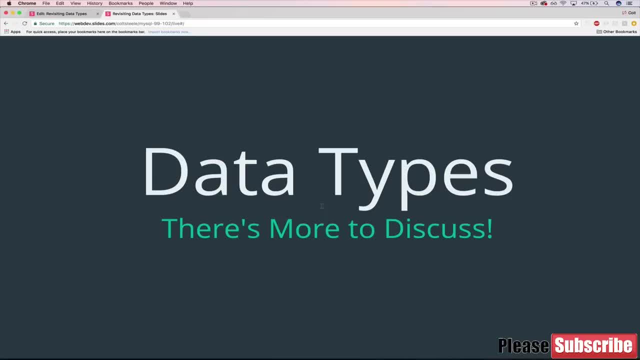 going to make a lot of sense. so we're going to focus on. what we're going to do is focus on what will have the highest impact for you. what has the highest impact in, you know, my developer life and the people that i know and have to talk to and about how they use my sql. so, basically, it boils. 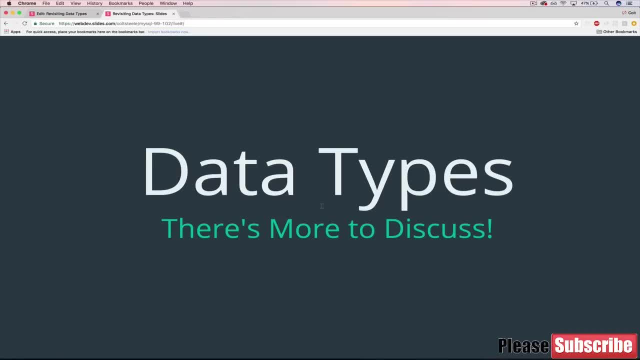 down to a couple different data types and a couple different broad categories. so the first category is uh, text or string data types, and then we'll also talk about numeric data types. we have a lot to talk about there, because we've only worked with ints we need to talk about. 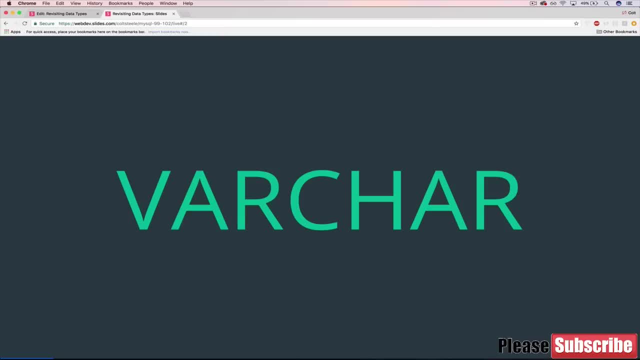 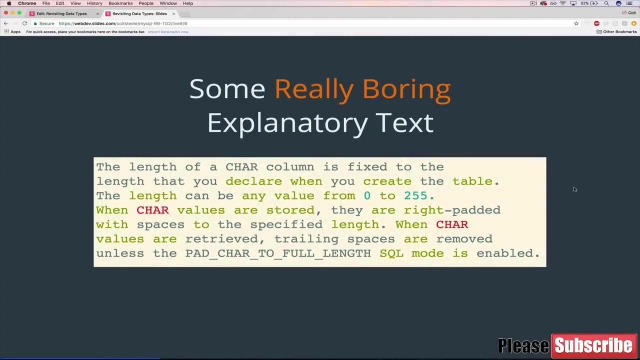 how we store decimal points or how we store, you know, non-whole numbers- can't remember the term for that- and also we need to talk about how we store things like dates and times. really important part of using a database is typically at least in web applications or applications in general. you're. 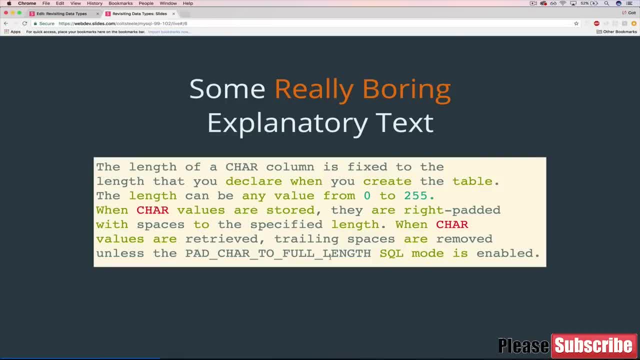 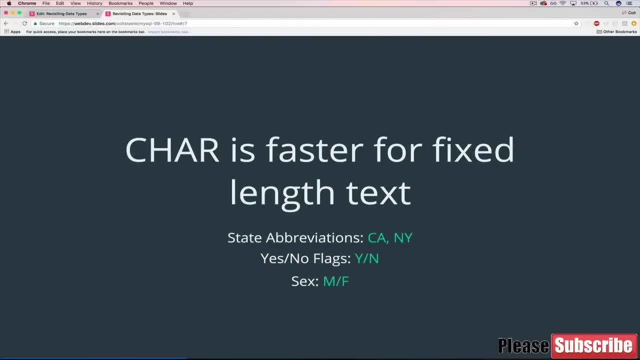 usually storing some sort of date and time information about when a transaction happens, when somebody signs up for your site, the last time something was updated, and so on. so we'll be talking about that in a little bit, but for now, in this video, we're focusing on storing text, so as 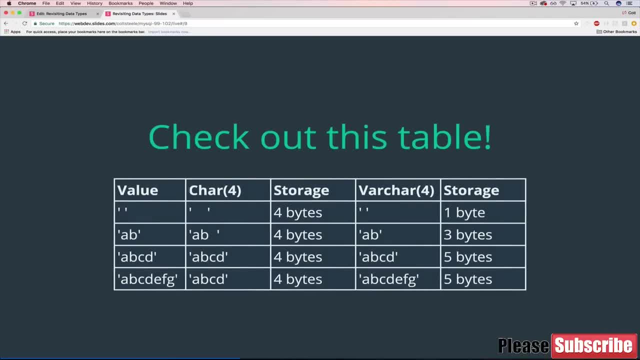 i mentioned, we've already seen varchar or varchar, however you want to say it. i think most people actually say varchar, but i don't know. i say varchar doesn't really make sense. i guess you say character, not character. all right, so we've already talked about it. it's what we've been using. 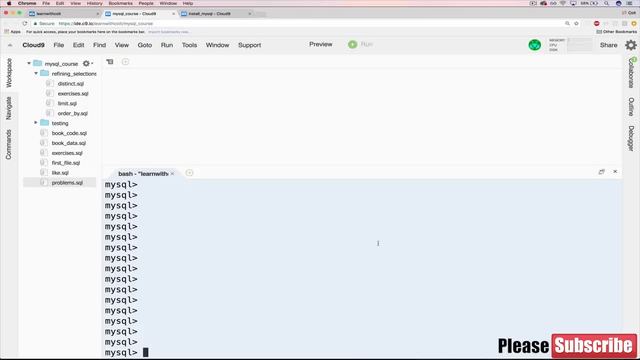 to store text, but there's also char or car, which is, uh, an additional type of text that we're going to talk about. looking at it, and it was a completely different, separate data type. now they both store text, but there's one really key difference. well, what is that difference? 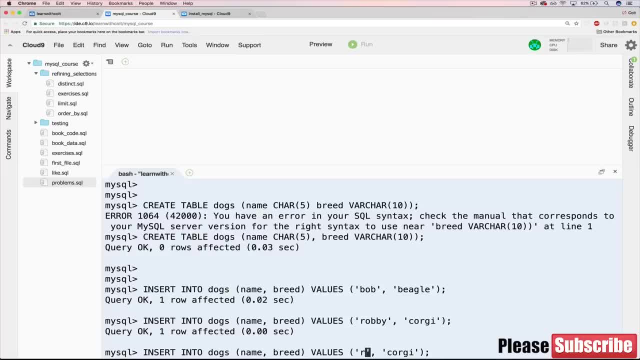 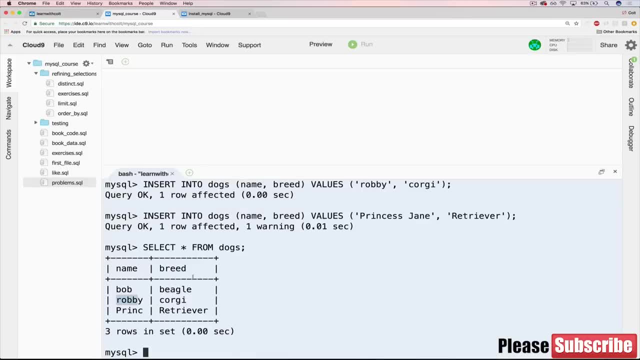 char has a fixed length. so when we specify, let's say we're working on, let's say we're working with our books table and we want to have a column called title. we could have right now it's a varchar in our existing books table, but we could specify it's a char. 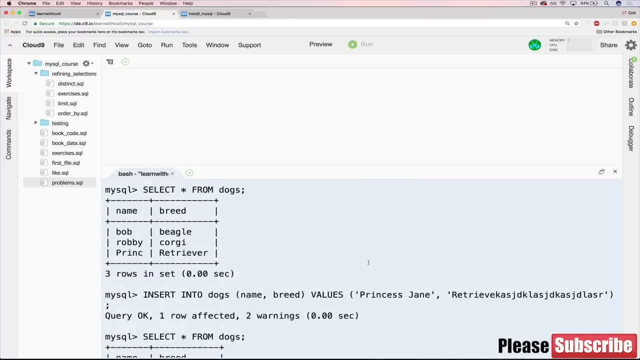 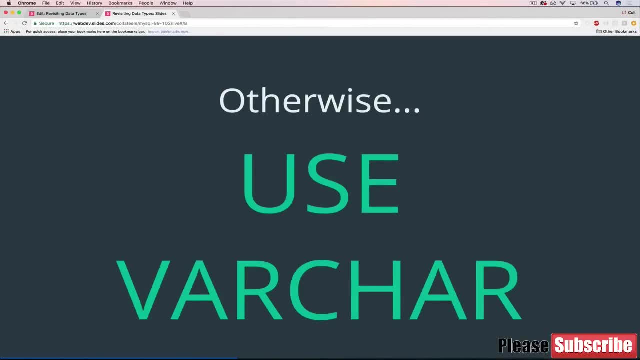 length of five for title, And what that means is that every title that we add in is going to be five characters. So if it's greater than five characters, if it's 10 characters, it's going to be truncated, It's going to get chopped at that five character mark And if it's fewer, you'll. 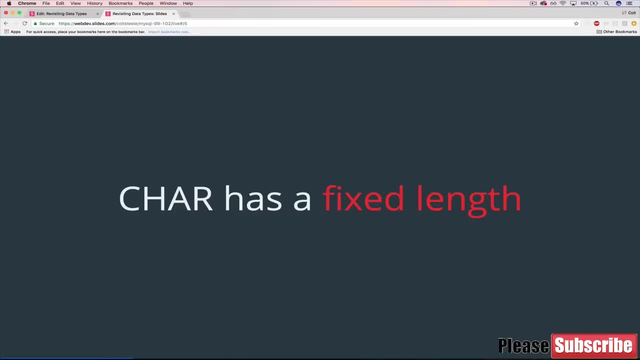 see in a moment what it does. It actually adds spaces to make it five characters. So char will always allocate the same amount of space for every row or every instance of that. char versus var. char can vary And, as you can see here, if we did something like char three, only three. 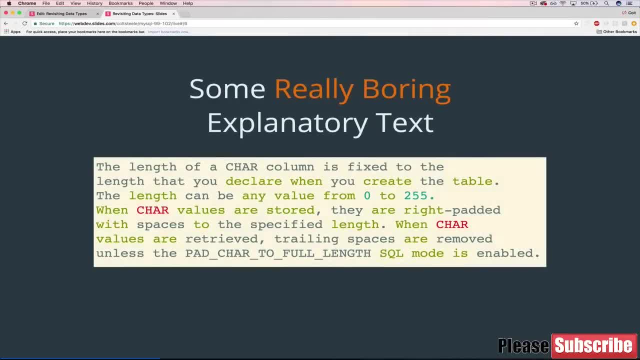 characters are allowed in this example. So this is taken straight from the documentation- some really boring explanatory text, but it has some important things to know. The length of a char column is fixed to the length that you declare when you create the table. We've already discussed. 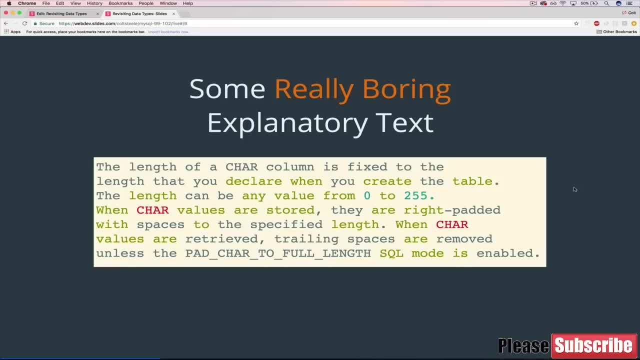 that The length can be any value from zero to two, five, five. So the longest char- char whatever- that you could have is 255 characters long. When char values are stored, they are right, padded with spaces to the specified length. 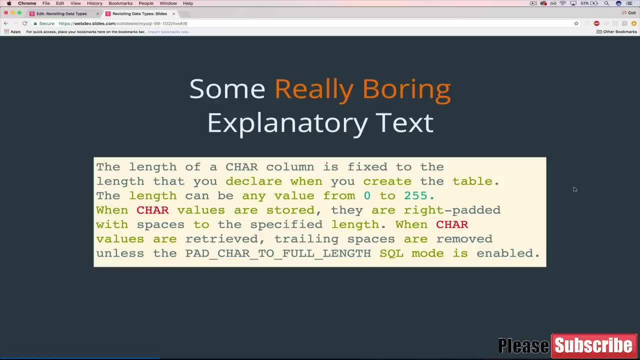 So that's kind of what I was explaining. If we have a 10 character limit- let's say char 10, and I, let's say I insert something that is only five characters, it's going to add five spaces after it, on the right side of it. pad it with these, basically: 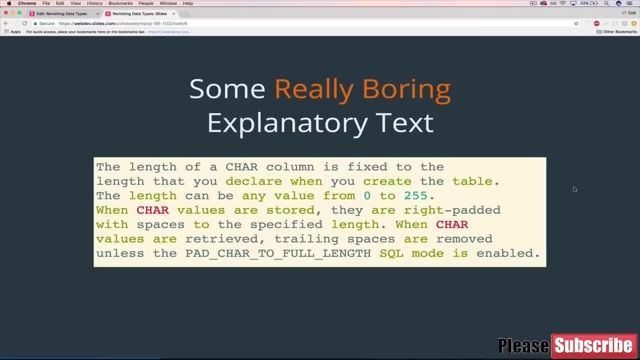 got just spaces to make it exactly 10 characters. However, it's kind of confusing because when you go to look at that string, when you select it back and it's retrieved, those spaces are actually removed. As you can see here, when char values are retrieved, trailing spaces are removed unless 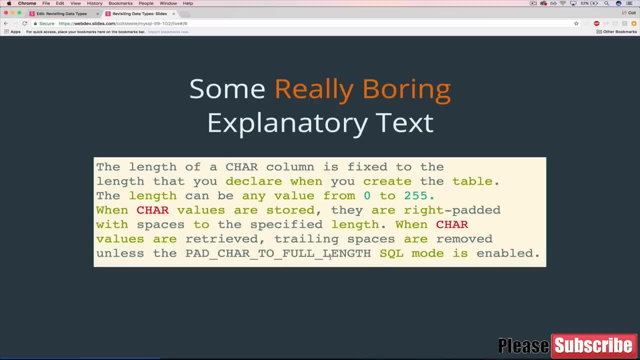 blah, blah blah. There is a way to get them to stay there, but I'm not sure why you would want that to happen. The only reason that I want to point that out is that I think it helps you, has helped other students that I've worked with understand how the fixed length works. 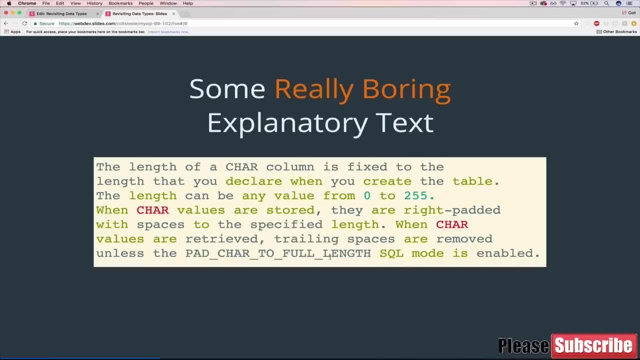 If you think in memory that it's actually storing something the same size every time. it's always five or always 10 characters and you can't get around that. So if you give it something shorter it will elongate it with spaces to make it 10 characters If you give 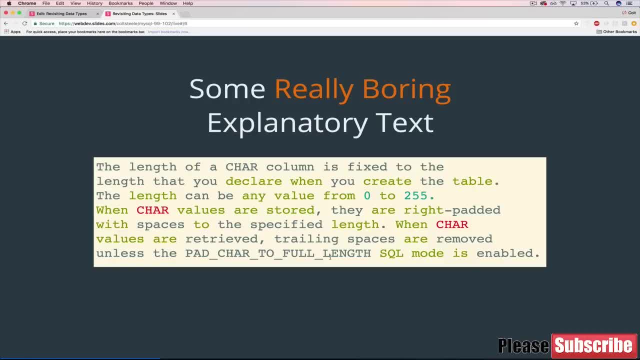 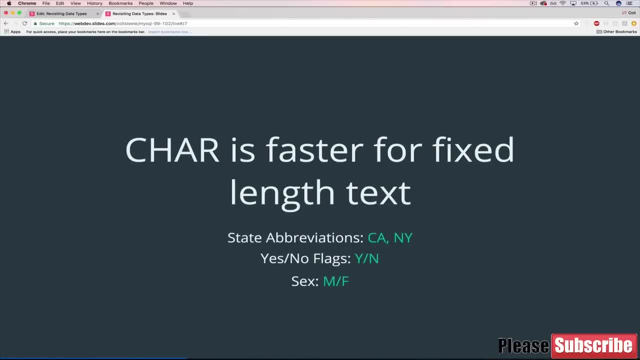 it something longer than 10 characters. it's going to truncate it to make it 10 characters, So why does it matter? Well, char is faster for fixed length text, So there's not a ton of uses in my experience day to day for using char, unless 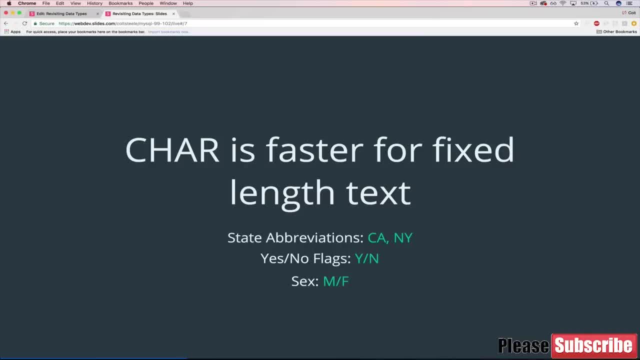 you know for sure that something is fixed length, So I tried to come up with some examples. like state abbreviations is one, at least in the US, where we have two letter abbreviations for every state. There's no reason to make that a variable length of our char. You can save space and time. 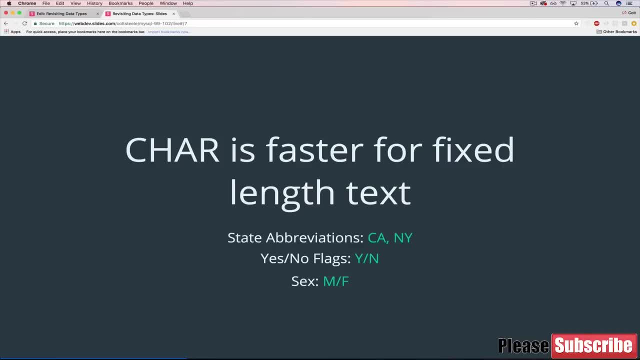 essentially by using char Or a yes or no flag, Y or N or any sort of like binary. it doesn't even have to be binary, but something that has a fixed length, So you could do sex in this case if you're doing where a pound or what do you call? 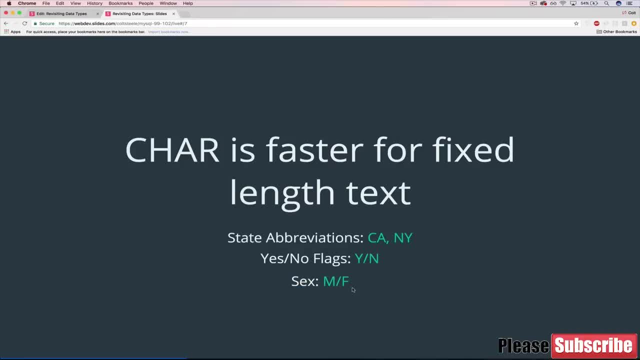 it an animal shelter. we're keeping track of animals and their sex- could use M and F. However, if we wanted to do things like male and female or unknown or whatever other options, those aren't all the same length, So it makes more sense to use var char. 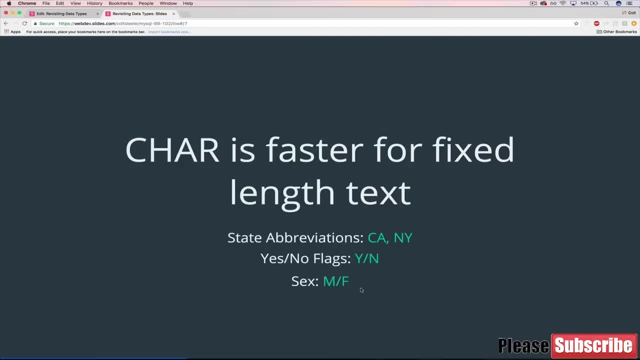 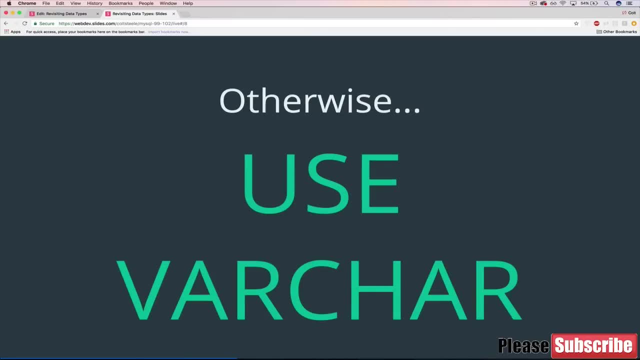 So you could probably come up with some other situations where this would make sense, But typically we use var char because it gives us a lot of flexibility. Otherwise, use var char. So there's a little. there's a table here that I actually took this from the docs. 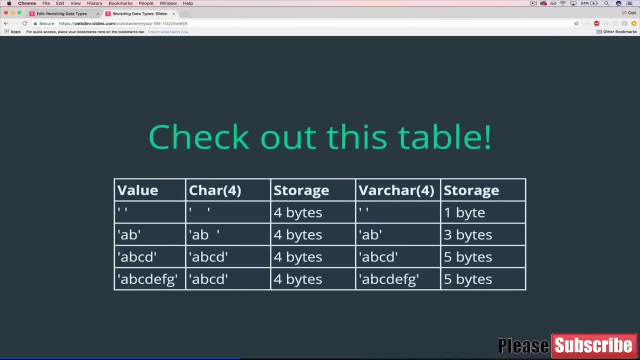 I just kind of blew it up and added it into my slides, But it's from the documentation for char and var char And what it's showing you here for a given value. like it, let's take a B, if we have a column with data type char four. 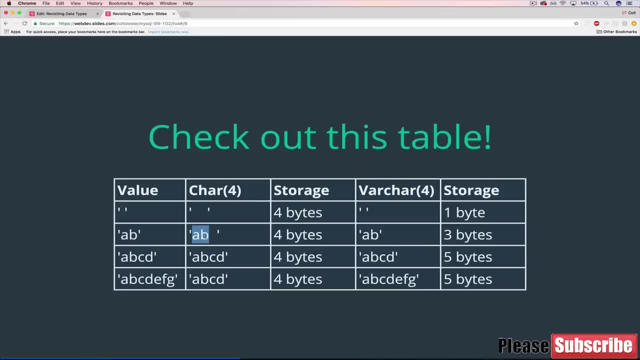 you can see that it adds the two spaces, So it's actually stored as a B space space. And if we store the same thing- the string a, B- in a column with var, char, four, so var char instead of char, it just stores a B. 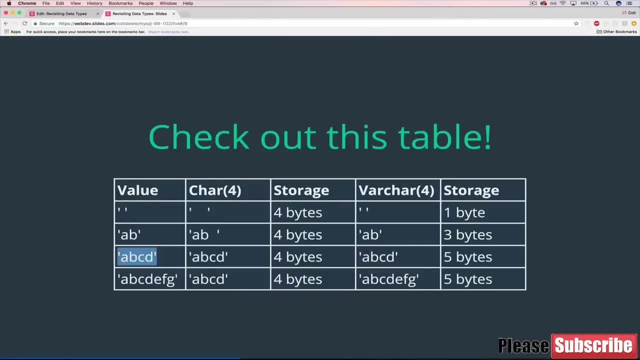 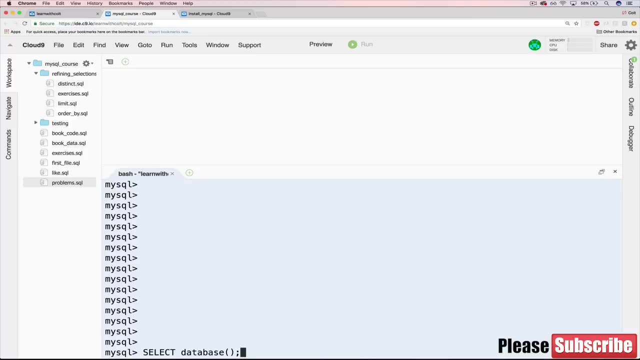 But what I want to call your attention to is not just how it's stored, but also the storage size, how many bytes it takes up. So if we look at char, when we declare char, for every single string that we insert into that column will always be four bytes, And you can see over here. 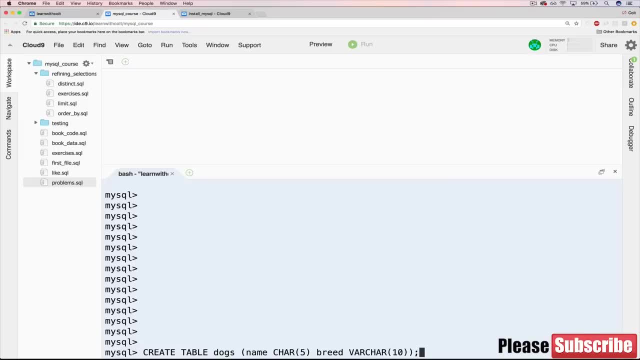 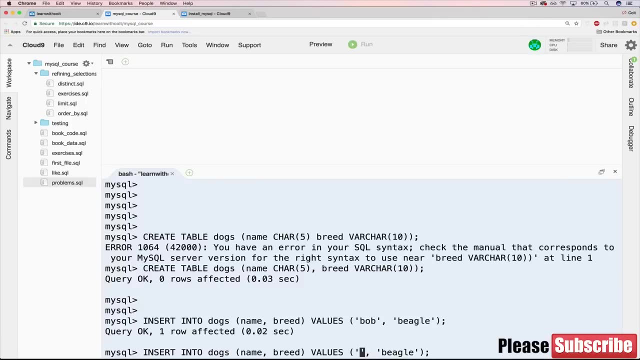 whether it's an empty string, it will convert it to be four spaces. If it's two characters, it adds two spaces. If it's four characters, it leaves it alone. If it's more than four, it truncates it. So we have a fixed size here. However, with the var char for 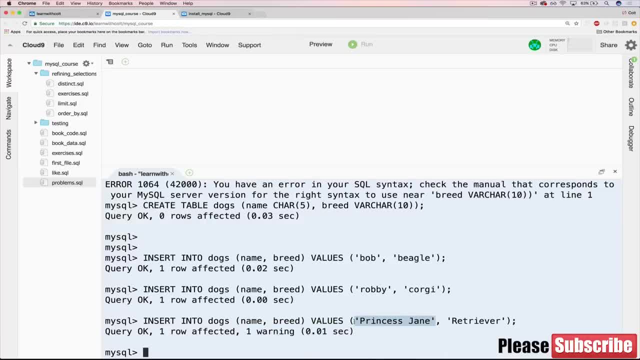 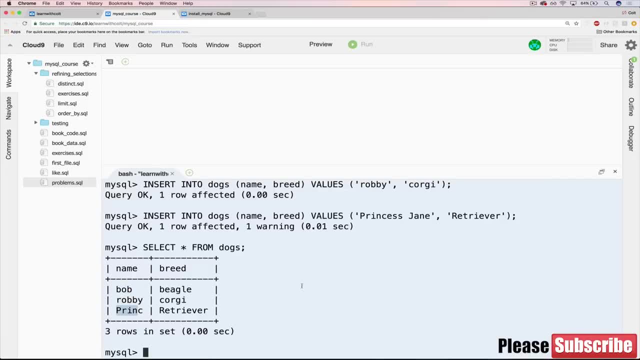 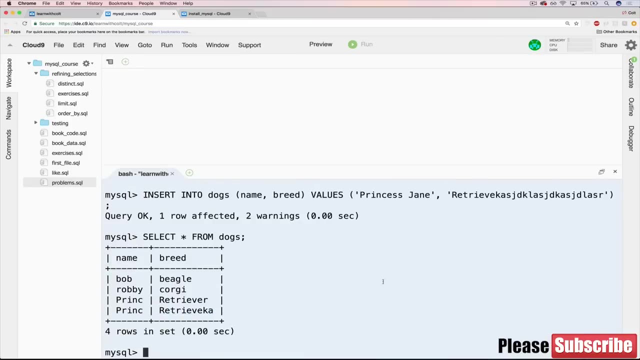 the same values, all have different storage sizes, So they're unchanged. when they're stored, We don't get spaces added, We don't get anything truncated, which is good, but you can see that our storage size does start to blossom. blossom, I don't know, starts to grow as the length of these strings grow. 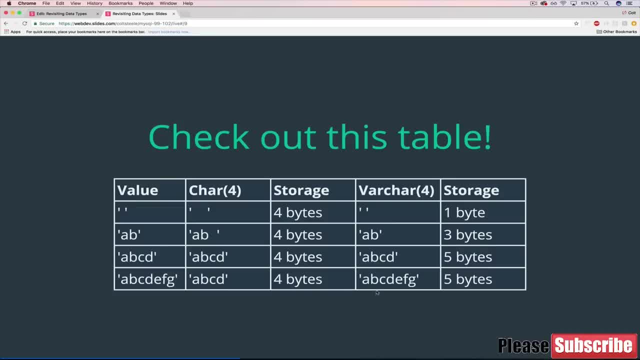 Now, it's not a one-to-one thing, So it's not like if we have a 10 character string here, it's going to take up 10 bytes, but there is a difference. That's all that matters. With that said, to be honest, that difference won't make a big difference. 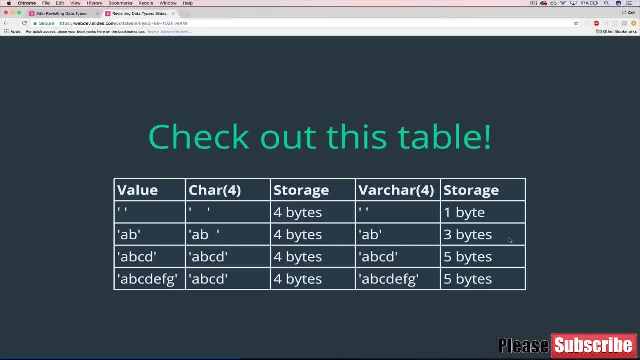 Let me put that another way. That difference is insignificant for most applications that I have ever worked on. If you are working on some giant app, you know you work at Bank of America and you've got, you know, tens of millions of customers and hundreds of millions of records. 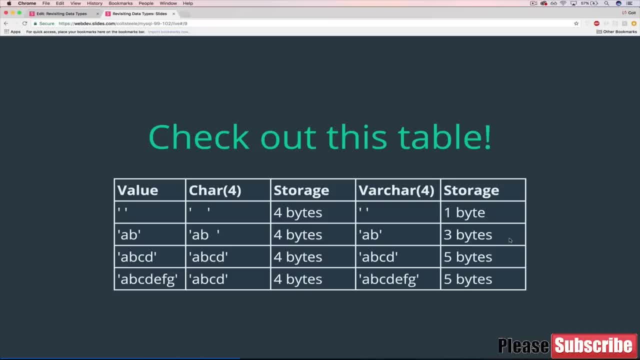 that does make a significant difference. But if you're working on a personal project or your own application, you don't really need to fret over this sort of thing. In fact it's. it's something sort of a common strategy that a lot of people would say is: just get something working And then. 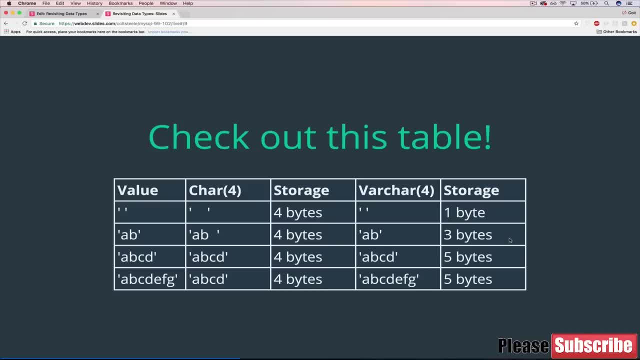 when you get it, when it comes time, you can optimize things. So if you start to realize, well, this one thing is becoming kind of slow, this query I'm writing, or whatever it is, maybe it makes sense for me to make this a fixed length and convert it to a char. Okay, So that's the 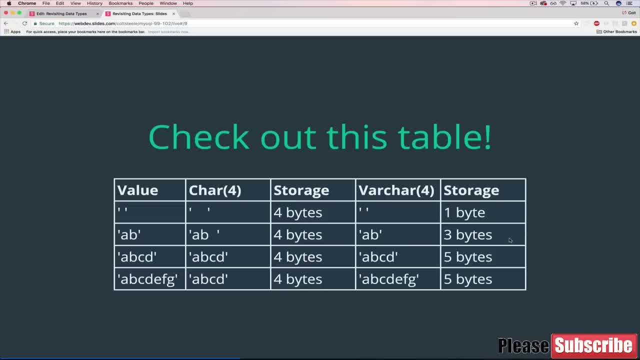 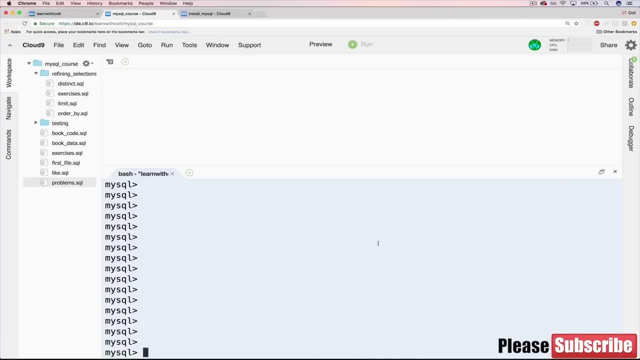 difference on paper. Um, you can go ahead. skip to the next video. I'm just going to show you in practice what it looks like. So I'm going to hop over to cloud nine And first thing I'll say I'm working in just a new database. I made, uh, basically just a. 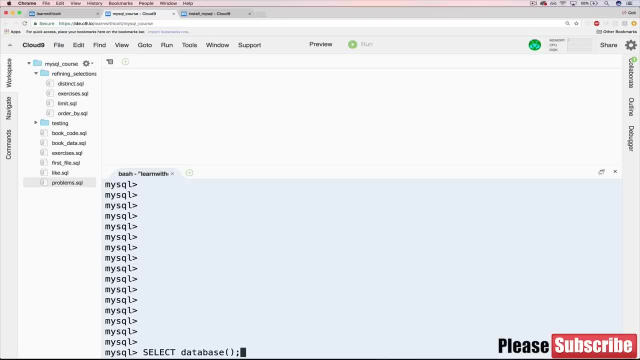 testing database. I didn't want to muddy the waters with our inside of our book shop database. I wanted to leave that alone, So I just made one called new testing DB. If you want to follow along, just make a new database. Hopefully you remember how to do that. Um, call it whatever. 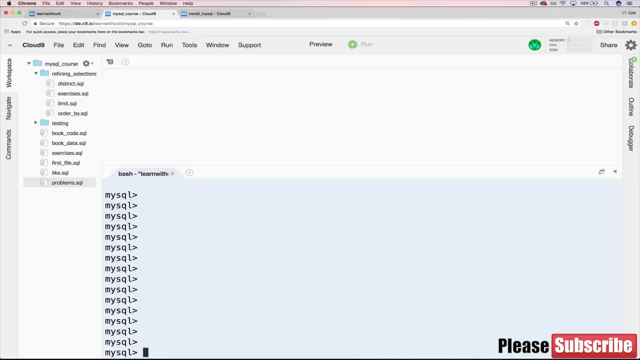 You want. I'm just going to delete it at the end of this anyways. So I'm going to create a table here, And all I want to do is have two different columns: One that's a char, one that's of our chart. 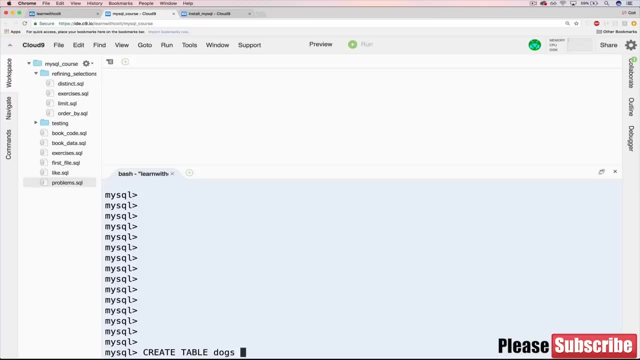 We'll just do dogs, Let's say create table dogs, and we'll have name, which will be char, a fixed length, five characters, And then we'll have breed, which will be bar char, And let's just say 10 there. Okay, Just like that, And we'll go ahead and hit enter. 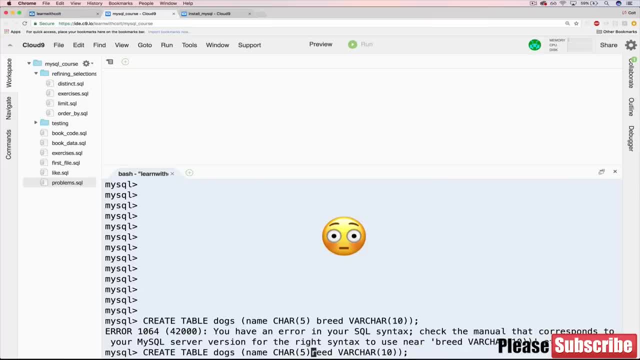 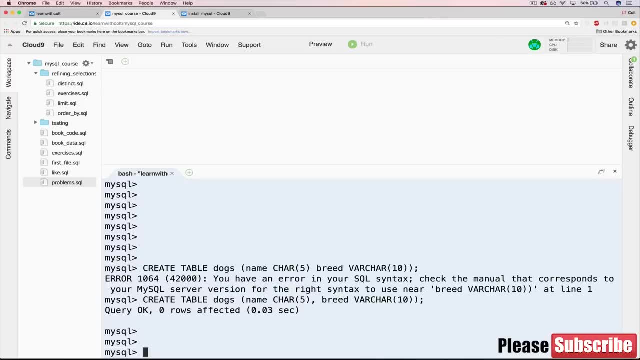 and I'm missing a comma. There we go. Okay, So we have that dog's table. Now let's insert some simple data. So the first thing that I'll do is insert into dogs and remember our syntax here. it's been a little while since we've inserted. we've been doing a lot of selects. 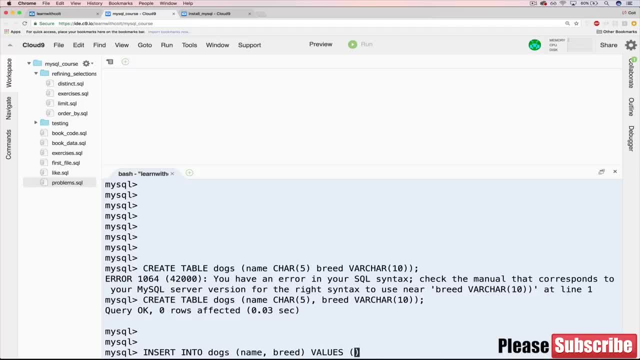 But we need to have our values and the values that we'll pass in. We're going to start with something that is less than five characters. So for name, let's say Bob, and breed will also be something short. Let's say uh well, what is a short dog breed? 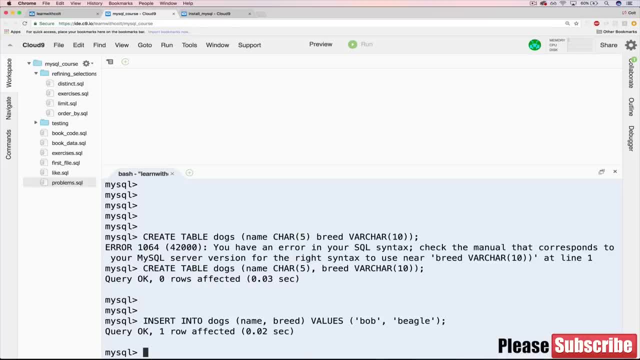 beagle, I guess, I don't know. Okay, So we'll do that and we'll do one more here. This time we'll have, uh, a name that's exactly five characters. Let's call it Robbie. spelled that way, I apologize. 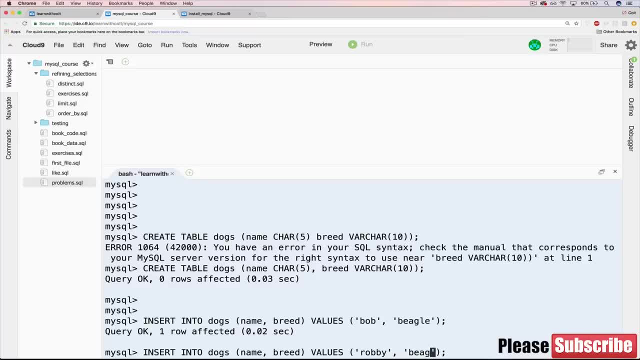 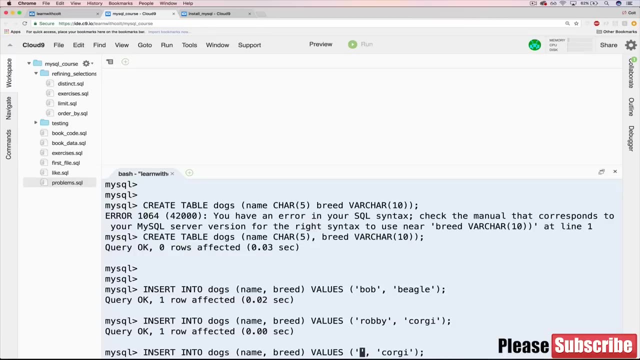 for unoriginal names here, Just trying to work with the constraints. Um and breed. here will be, uh, Corgi. Okay, And we'll do one more, And this time we'll have a long name. How about princess? 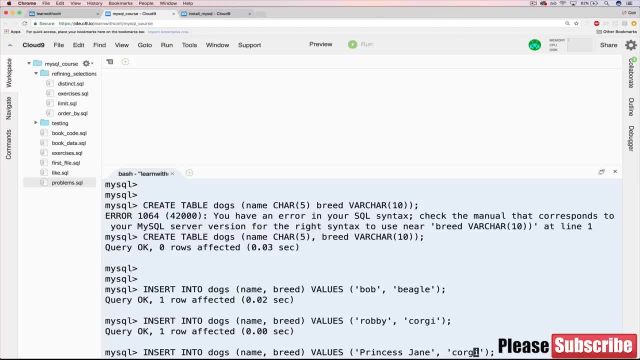 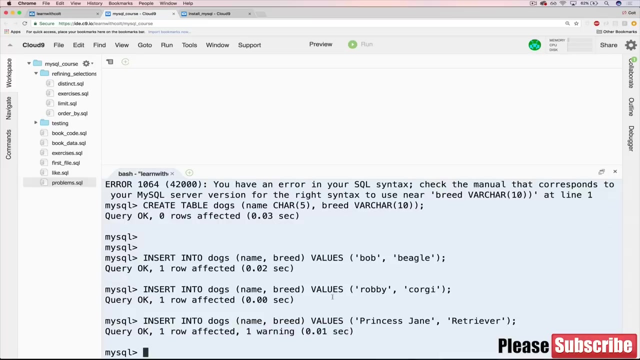 uh, Jane, and princess Jane is a man. I'm totally at a loss here. What's another breed? Let's go with retriever. I spelled that, right, Never remember. All right, Forgive me if that's spelled wrong, Okay. So first thing, first, right off the bat, notice: we got a warning on this last one. 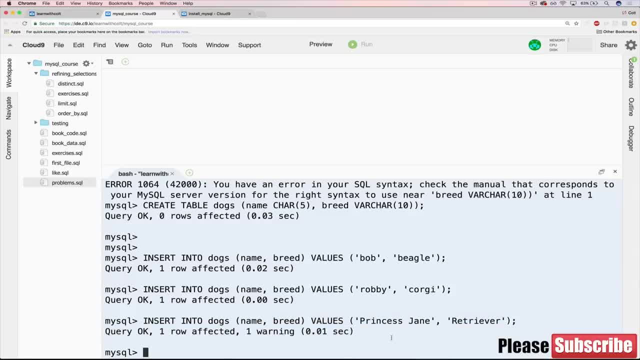 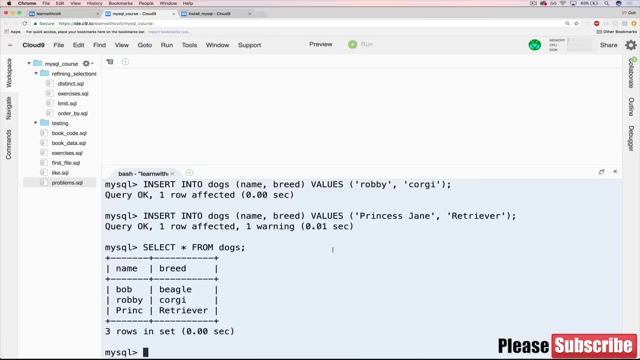 Why do you think that happened? Well, it's because princess Jane exceeds the limit that we've set for our char, which is five characters. So now, if we do a simple select star from dogs, you'll see we have Bob Robbie. they look good, They look the same, unchanged, And princess Jane. 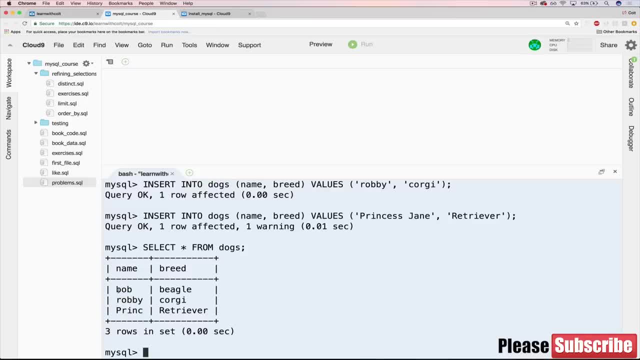 unfortunately, has been truncated. So, unfortunately, we can actually tell that there are those trailing spaces. Uh, because they're all trailing spaces, They're all trailing spaces, They're all trailing spaces. Uh, yeah, Uh, I have a little bit of trouble with this. Uh, at the moment I'm not. 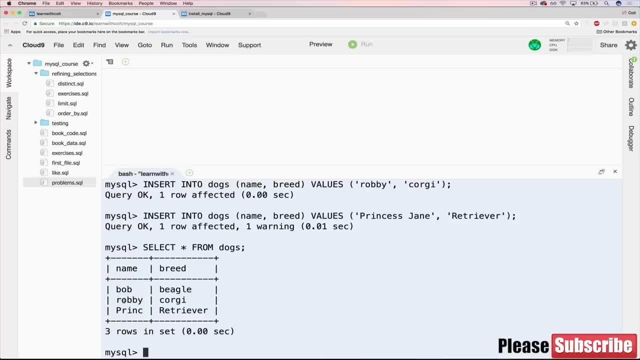 sure which one, because I'm trying to figure out what it is, But anyway, we'll see how long it will tell they are not actually here when the text is retrieved. remember what that giant bloater text said? it said that, uh, they're stored with these two extra spaces in our case, because this is three. 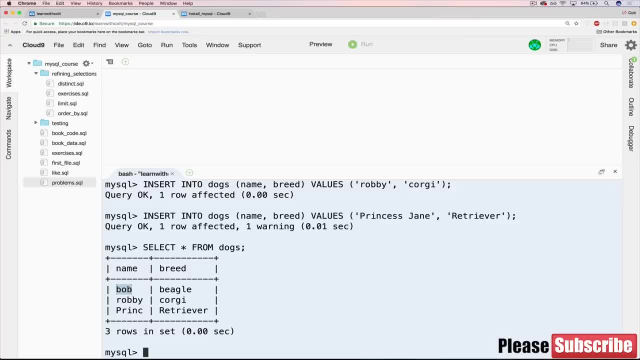 characters and we set up a five character fixed char. so they're in memory, are going to be two spaces here, but when it's pulled back out and displayed to us they're chopped off. um, robbie is unchanged because robbie is five characters long. princess jane, unfortunately, is cut off. 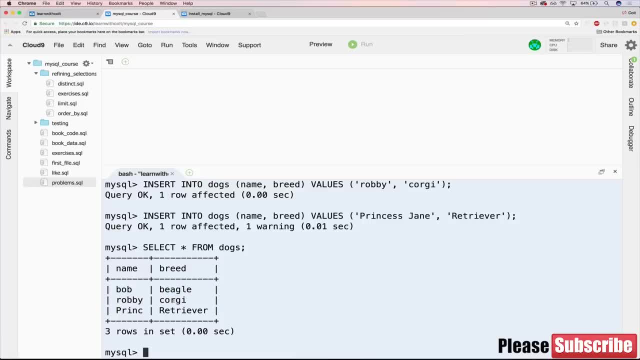 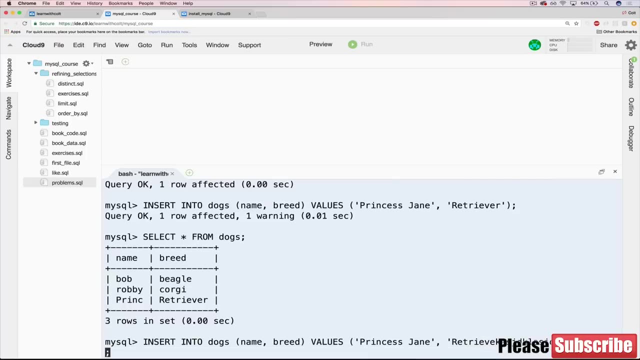 however, when we look over here, beagle corgian retriever varchar works how you expect. it's a variable character length. let's just do one more example here with princess jane. yeah, we'll just have another princess jane and a long retriever, blah, blah, blah, blah, blah. now, when i do a select, 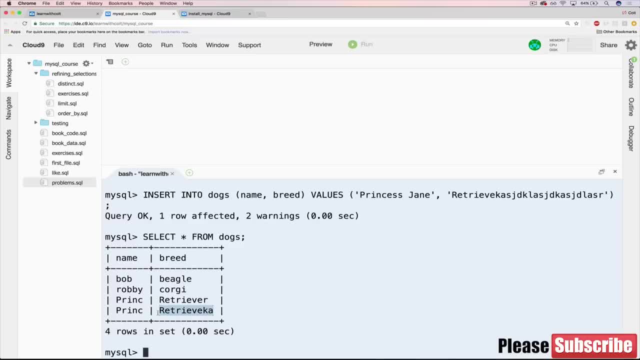 star. notice again what happened. this is what we expect to happen. we've already seen this. how varchar works you? it still has a maximum length that we can provide. in this case, we did 10, i believe. yes, um, so it can work similarly to a char in that state in that sense, where it will truncate things. 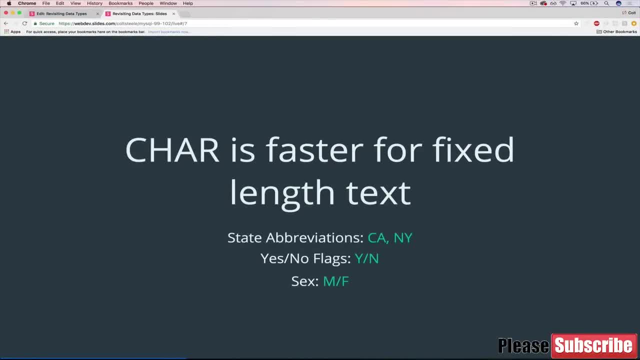 so just to wrap up the end here, char again is faster for fixed length text. so if you know something is always going to be the same size, use char. however, if you have any doubt, use varchar, and again the difference is relatively small. so if you know something is always going to be the 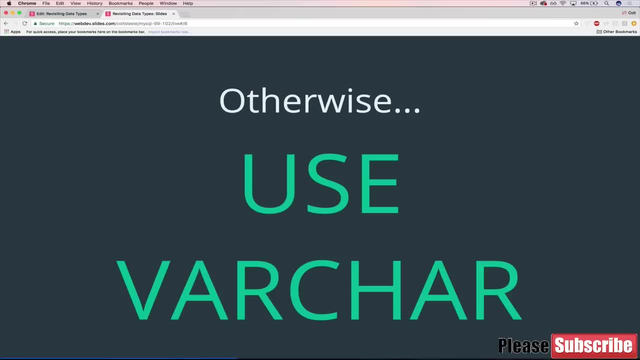 same as you did earlier. yes, pressing index does not need to be an integral field. this is relatively insignificant for most of the things and i don't want to be presumptuous, but most the time it's not going to be a deal breaker. okay, so moving on. we're now going to discuss numbers. 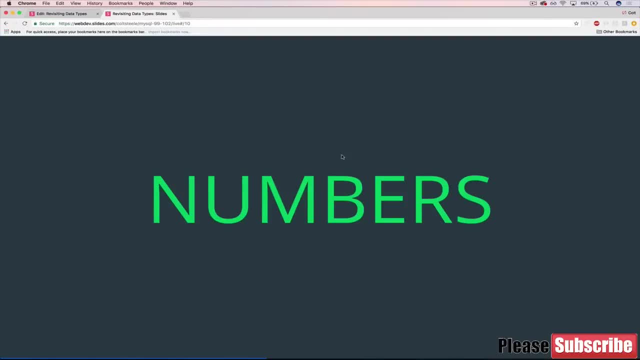 in the next video, not this video. okay, so next up in this onslaught of data types, we're going to discuss some important numeric types. so there are quite a few. uh, we've already discussed Int. we've used it quite a bit. it works with whole numbers, so it's useful if you're working with. 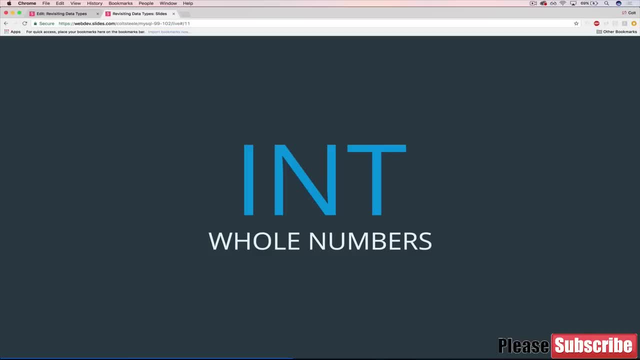 things where you need them or want them to be, whole numbers where decimals don't matter. so we know how it works at this point. however, there are a bunch of other data types that mysql comes with. we're not going to talk about every single one. we're just going to talk about the ones that 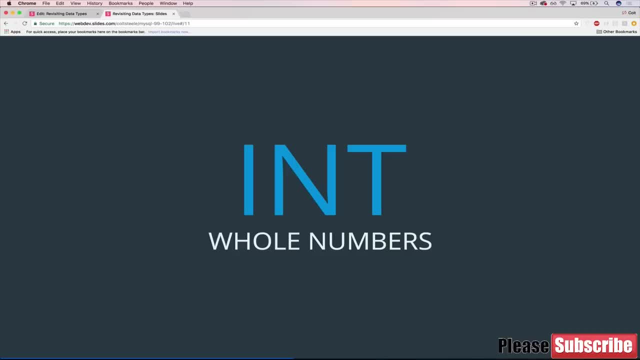 will matter the most, and in my opinion those are. the first one is decimal. so decimal is what it sounds like. it's a number that includes a decimal afterwards, or how can i put this? i don't think that's the right way of saying it. it's a number that includes a decimal point and something after. 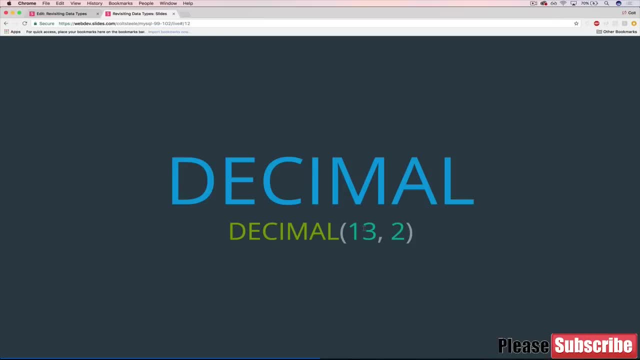 it, or it can include something after it. so when we create a column, we actually provide two arguments, and we'll talk about those in just a moment. but the important part here is that it's a way of creating a column that will store numbers that include decimals, something after the decimal point. 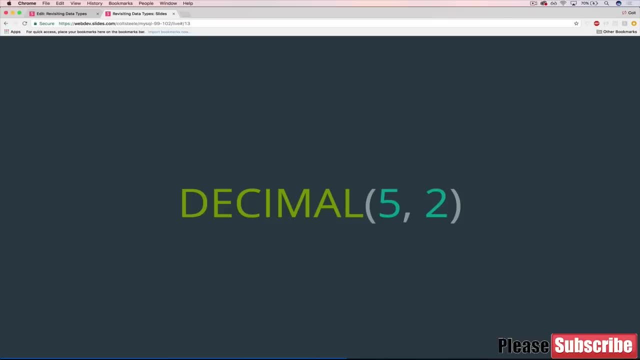 so what are these two numbers we're passing in? well, on this next slide, have a handy little graphic here. when we run or when we create a column, let's say: let's call it price. this is a price of a i don't know. let's work with books or books price. we have two different. 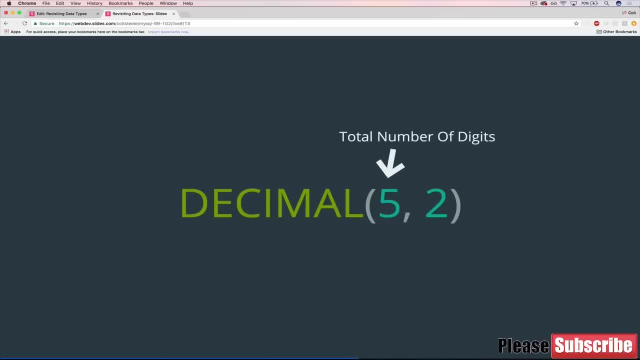 arguments. the first one, five- tells mysql the maximum number of digits that our number can have. so that actually includes both before and after the decimal point. and then the second number is how many digits count. I'm after the decimal point, so another way of looking at it something like this: here's the 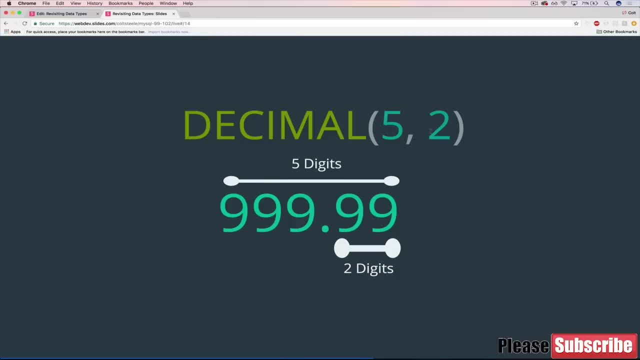 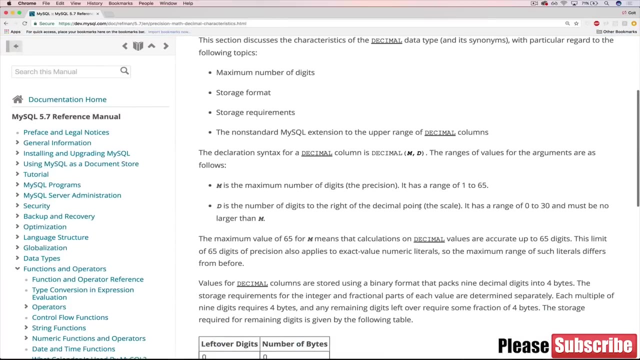 maximum number we can store in a decimal, five comma two, so it's five digits long. two of those digits are after the decimal point and if we hop over to the documentation, which I'll try and hold my tongue but I definitely find to be occasionally subpar. 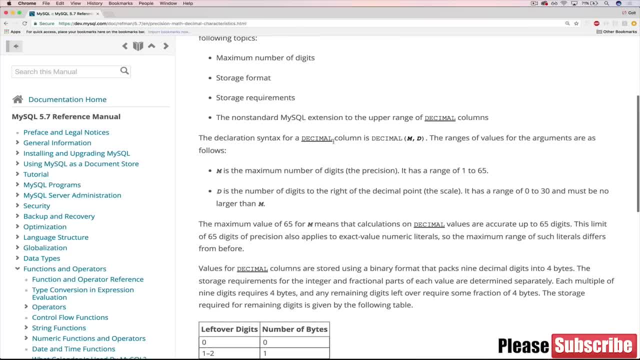 it does an okay job here explaining it. so the declaration syntax for a decimal column is decimal m, comma d. m is the maximum number of digits. the precision it can go up to 65. d is the number of digits to the right of the decimal point, also called the. 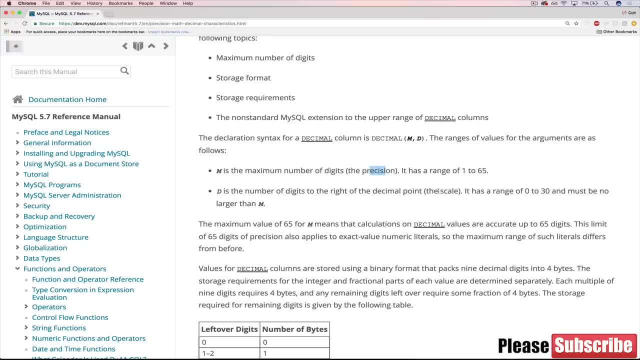 scale- I have never heard anyone actually use those terms, but I guess it's good to know- and it has a range of 0 to 30.. so there can be no more than 30 digits after the decimal point, which in most cases is going to be plenty. 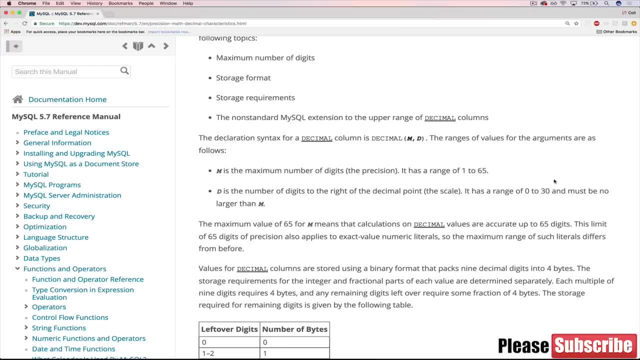 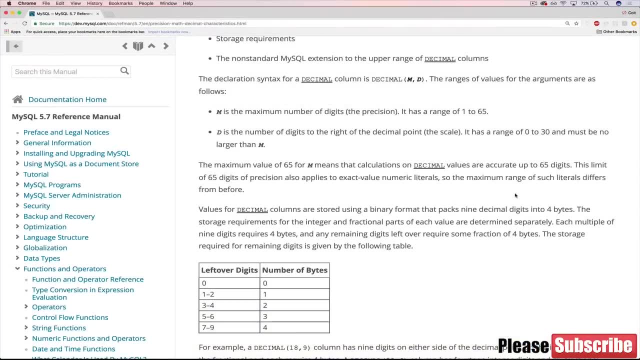 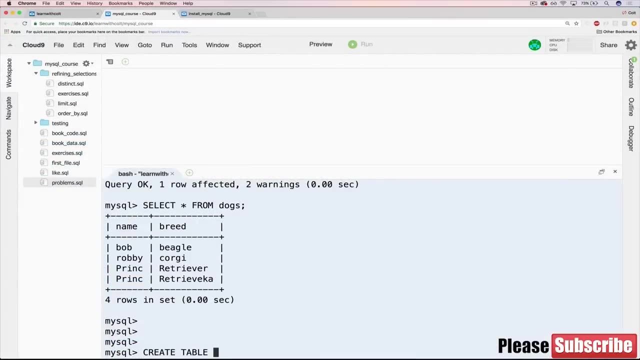 I mean way, way, way more than you pretty much ever need. so this that's the gist of decimal here. it lets us store numbers that are decimals, but we do need to specify roughly what those numbers need to look like. so we'll create a very simple table, let's say a generic. 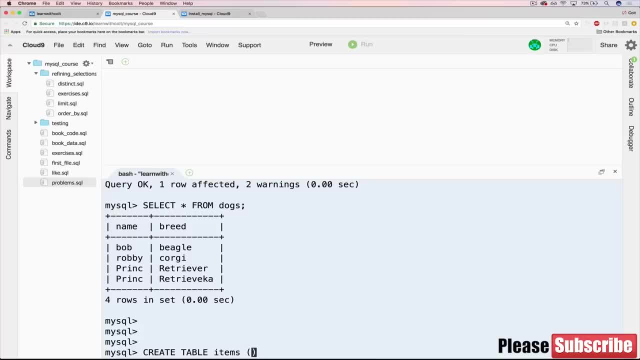 item. so items, and all we're going to have is a price. we won't even worry about a name or anything. so we'll have a column called price, which is a decimal, and let's go with what we saw there: five comma two, just like that. okay, so we have that. now let's insert a couple things and test it out. 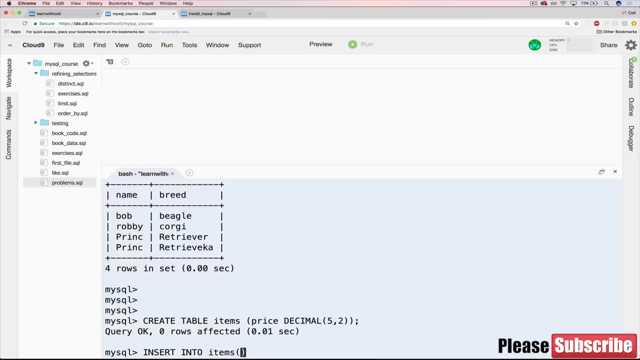 so insert into items the first one that we'll do what we need to specify price and then values, and the first one will be just a whole number. let's say seven, just like that. okay, then let's do a long, whole number like that. see that we get a warning. then let's do 34.88. 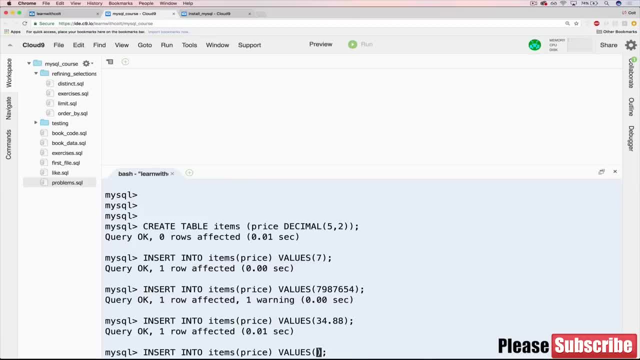 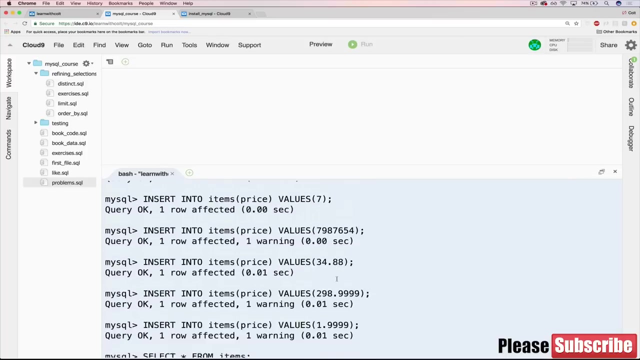 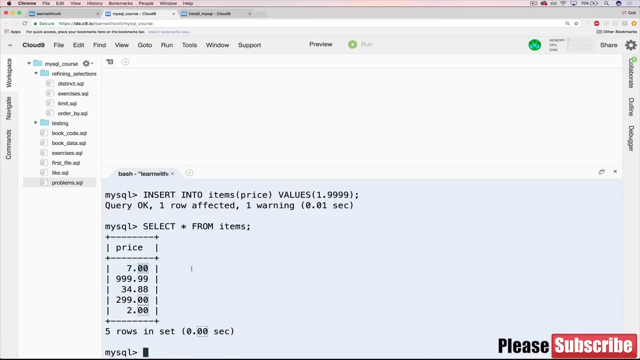 then let's also do a 298.9999 and finally let's do 1.9999. okay, so now let's do our select star from items and see what we have. okay, so the first thing that you'll notice is, when we inserted seven without a decimal, it added those two decimal places for us. 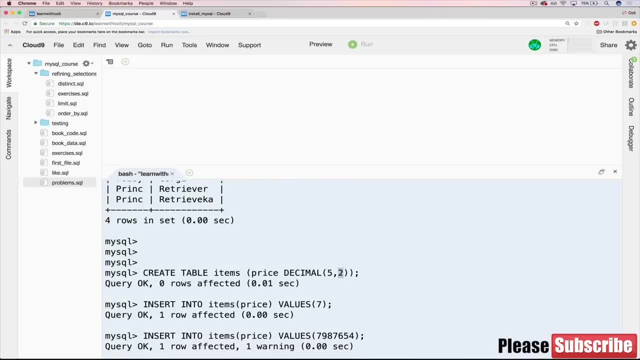 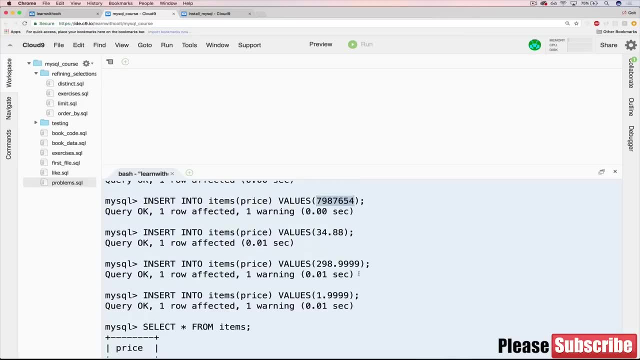 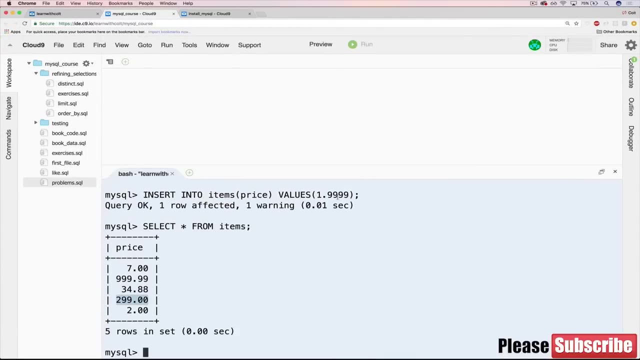 and again. that's because when we created the table we said there are two places after the decimal, so it adds those in, even if it's a nice whole number. this next one is a bit weird. we never inserted 999.99, we inserted 7987654. 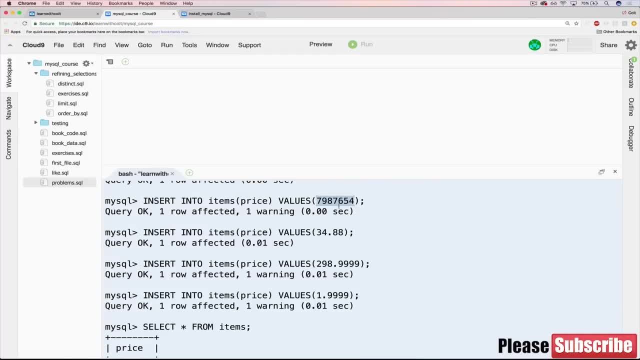 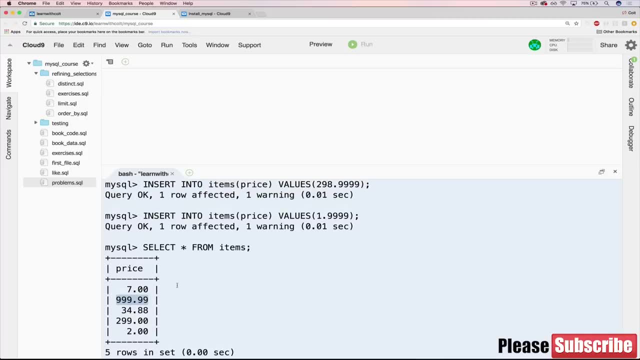 so what's happening here is that this is much larger than the maximum number allowed. the maximum number allowed, as you can see here, is 999.99, because we specified it's five digits total, with two coming after the decimal. so that gives us 999.99. so good to know when you do this. if you 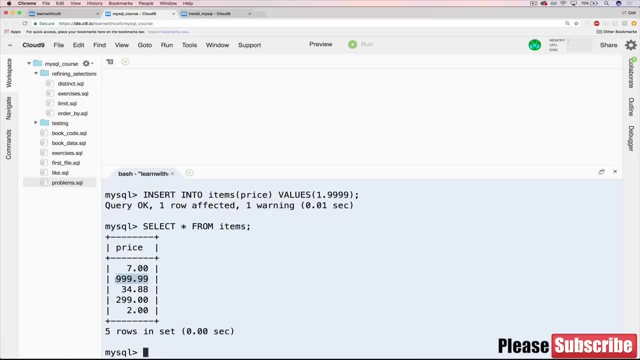 oil a number, for example act times, in order to integrate a number that's too large, it's going to just put the largest possible decimal, given the constraints you set up. then, next up, we have our 34.88, which looks just the same, and then we have 298.9999. 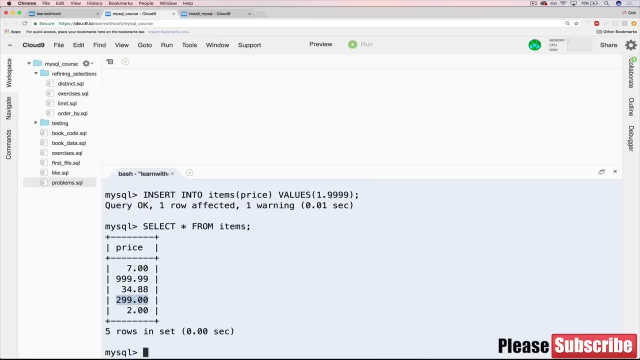 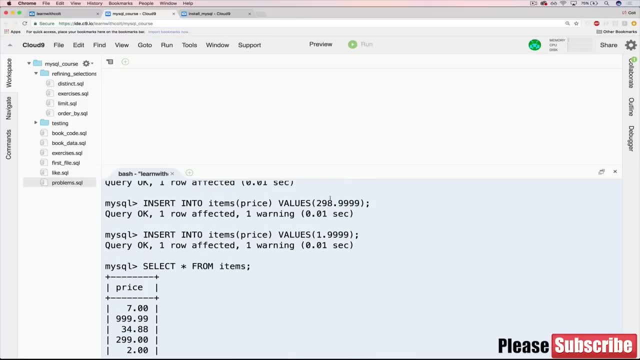 which you'll notice here is actually rounded up, so it's rounded to 299, and that's because we specified rounding to two decimal places and when we do that, Well, actually it's on this one. here It will round up to 299.00.. 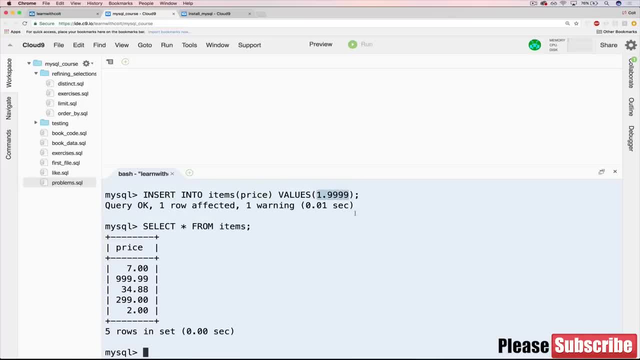 Same thing applies here, where we have 1.9999.. So that's the basics of the decimal data type Pretty commonly used. I'll be using it throughout the course. With that said, there are other data types that we can use to do the same thing. 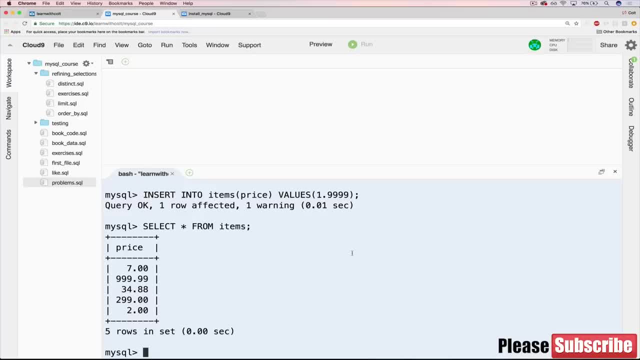 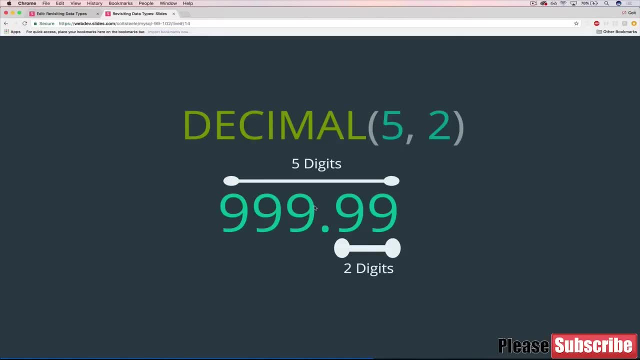 that we're going to talk about in the next video, and we'll discuss why and when you would use each one. Okay, so we discussed the decimal type and you've already seen the int type, but we're focusing on the decimal type, or we did focus on it. 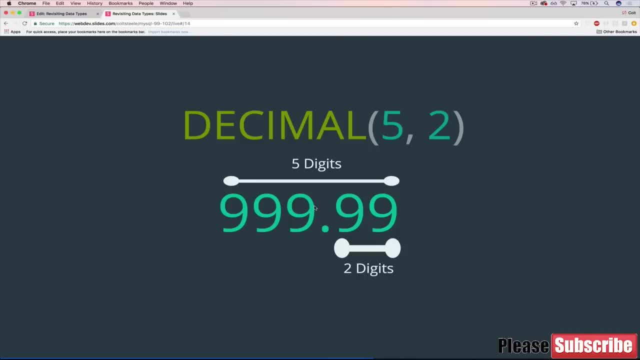 But, like I said, there's a bit of competition, So there are other types that we could use to represent similar data, which is to say, numbers that are not whole numbers. So there's also things like float and double, So we're going to talk about those in this video. 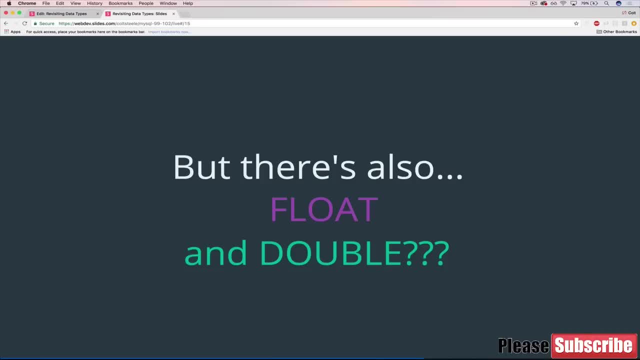 The differences- I'll have to be upfront- between all of them are are quite technical. They have to do with how things are stored in memory. It would be difficult to explain, without going all the way into, how binary works and base 10 versus base two, and how things are stored in memory. 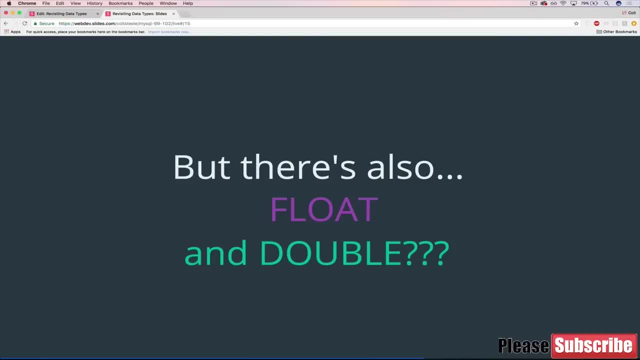 So I'm going to kind of skim over some of this, because the honest answer is that it doesn't, or the truth is that it doesn't really matter. All that matters is that you know functionally what the difference is, But if you do want to learn more about the difference between them, 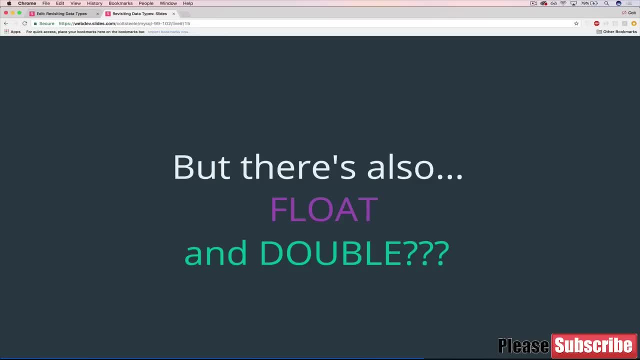 there are some Good resources online And I highly recommend that you check out some YouTube videos, and I would love to link you to a specific one. However, I've had some copyright claim issues, So last time I did that, I'm not going to do it. 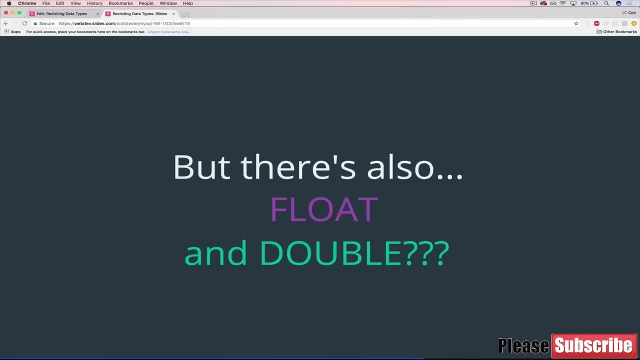 Now, if you're curious, you can research it. Uh, but essentially it, like I said, it boils down to how they're stored. So the big question is: what is the difference between float and double? Let's take them as a unit and decimal. 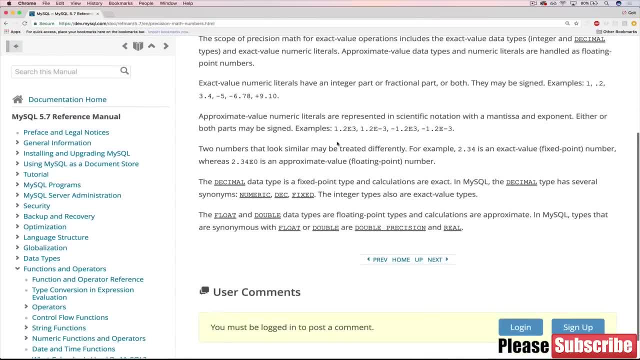 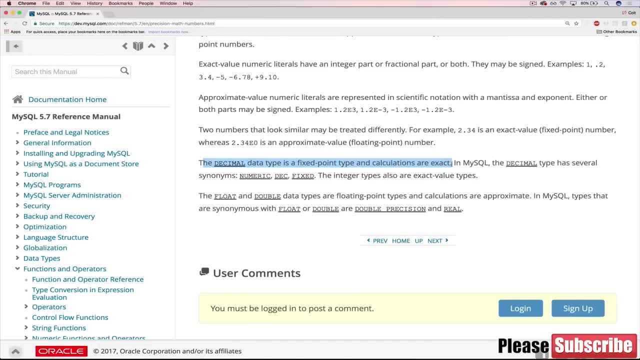 And if we go to the documentation, there's a page that lays it out Relatively plainly. it says: the decimal data type is a fixed point type and calculations are exact. The float and double data types are floating point types and calculations are approximate. 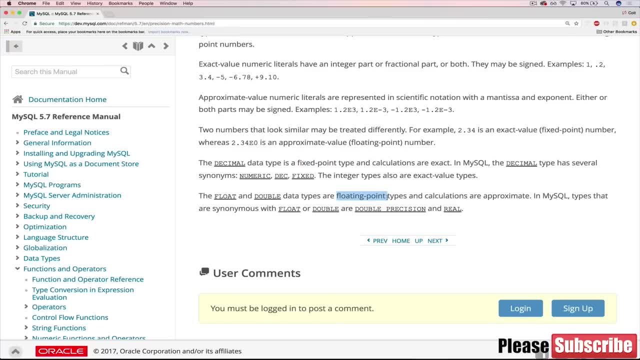 So we've got fixed point and floating point. They are different. That's. that has to do with how I, what I was describing, how they're stored in memory is different. Um, that's not as important. Just knowing that they are different is important. 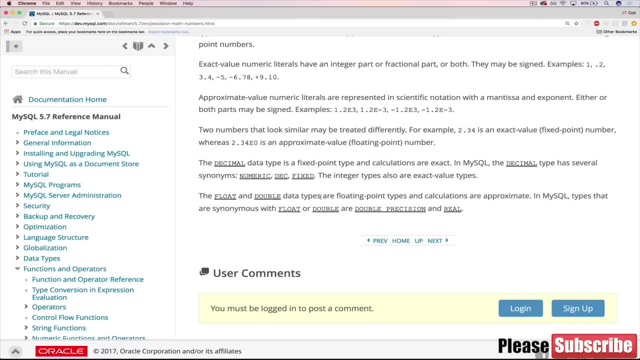 However, the side effect of how they're stored is that float and doubles are approximate, which seems kind of weird. Uh, it doesn't seem like you would ever want to use them if they are not exact. Uh, but it essentially they're approximate and decimals are exact. 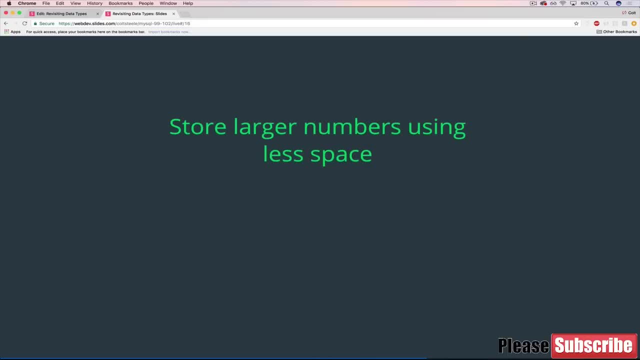 So, to boil it down, float and double will store larger numbers using less space. So that's an advantage. They can take gigantic numbers, things that you can't store in a decimal, And they'll use less space. However, that comes at a big cost. 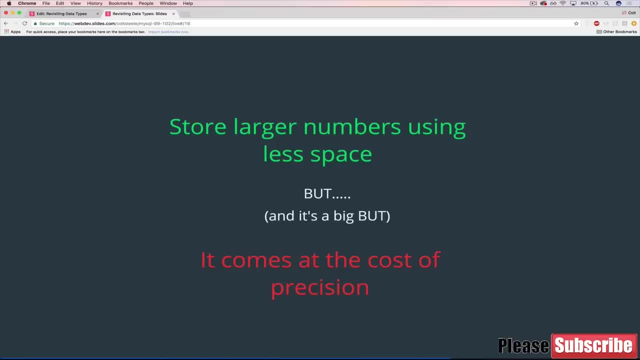 It's a big, but it comes to the cost of precision. So it doesn't mean that your numbers will be wildly inaccurate if you're using a float or a double, but it does mean that they're not going to be as accurate as a decimal. 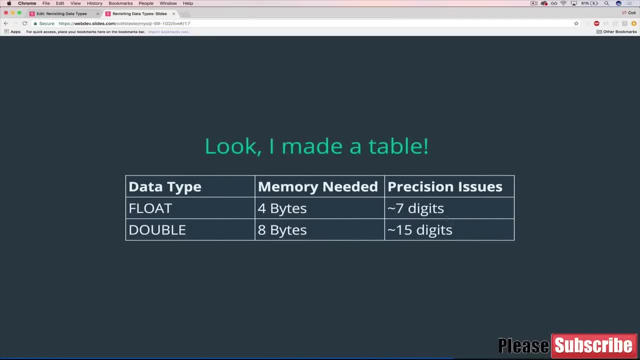 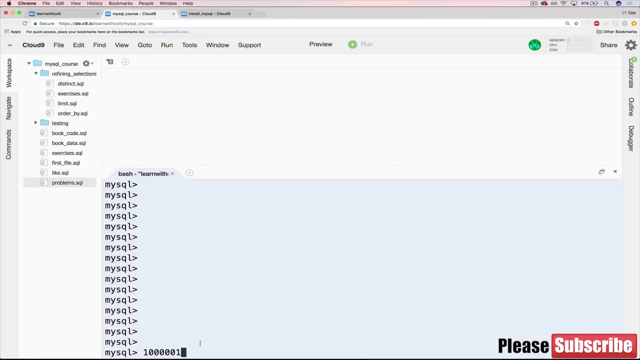 So here's a simple table that it just basically takes information from the documentation. Floats will have precision issues After around seven digits, So if we had something like this number here, we could run into a problem where this one might not reliably be one. 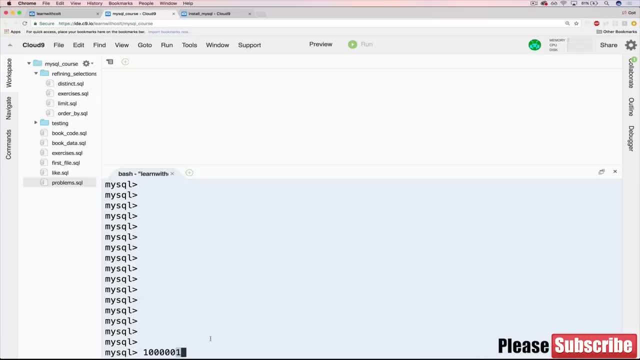 When we retrieve it, it might change, Um, and that could be problematic if you're needed to be precise, But if you're working with gigantic numbers, something like this, or let's even add in something like this, this one at the very end. 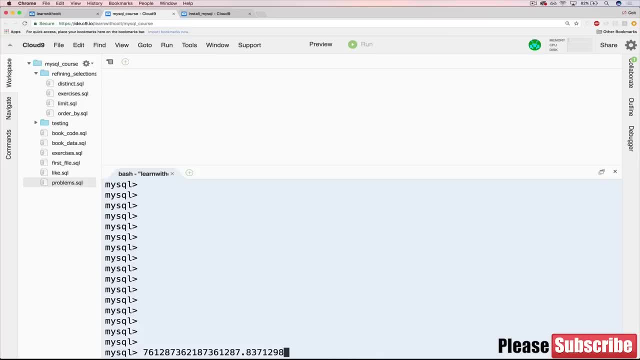 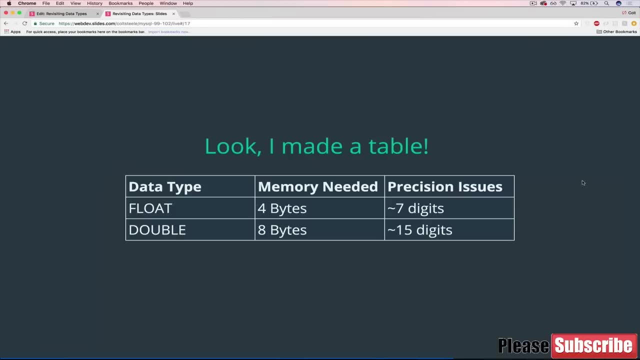 isn't going to be a deal breaker most of the time, depending on what you're working with, Um. with that said, it's really important to know that there is a difference And there's a lot of kind of classic bugs and issues people have run into lots of blog posts around floating point. 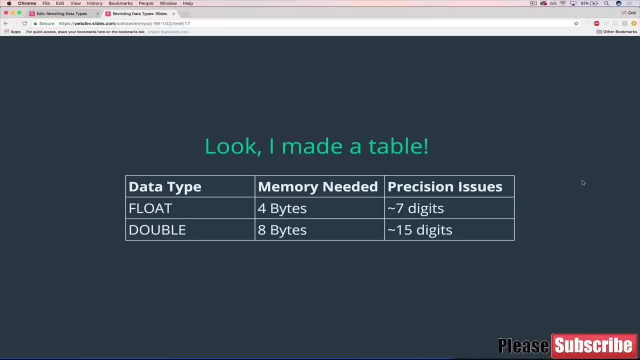 math problems, floating point, math issues and bugs. doubles are basically the same thing as a float. They're just bigger. They have larger capacity. However, they take up more space in memory. You can see four bytes versus eight bytes A double. 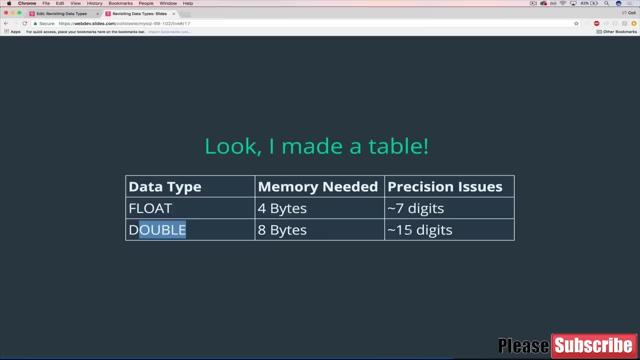 however, is more precise. so it's precise to roughly 15 digits rather than just seven. So if you do use one of these, it's better to use double, which brings us to the question: what numeric data type should you use when you're storing information that has a decimal? 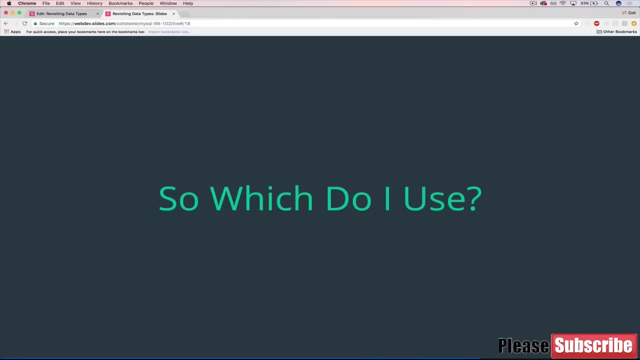 And the answer, at least in my opinion, is you should always try and use decimal unless you know that precision doesn't matter. So if you're doing things like financial data, prices, if you're a bank, you need that precision. 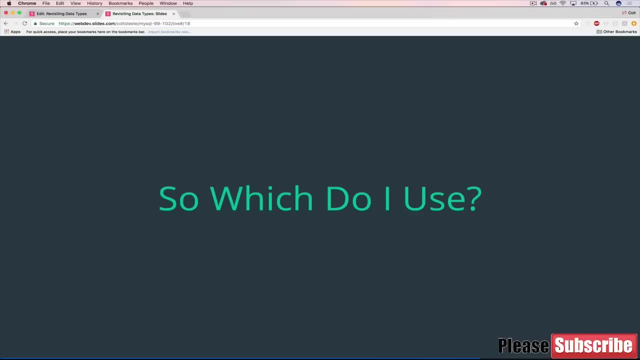 Absolutely, You need to use decimal, Otherwise you can get away with floats or doubles, But for the most part I'll be using decimal. It's kind of my preferred data type when we're working with decimals. Oh, and before I forget, 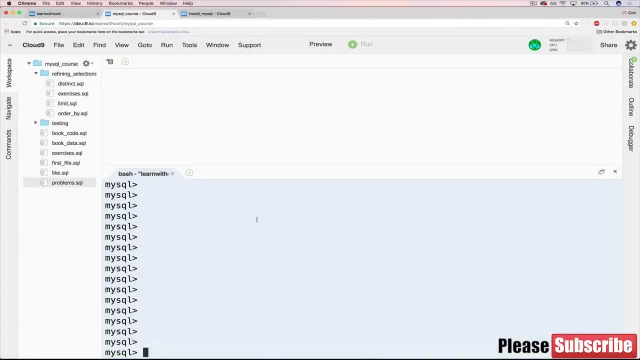 well, actually I already forgot, but this is after I recorded the video I'm going and adding this in. I wanted to show you. You can actually see the inconsistency, the impreciseness of using floats and doubles as well. 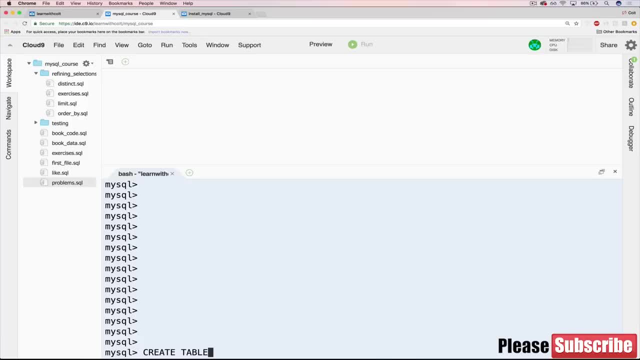 So I'm going to create a simple table and I will just call it um, let's go with thingies. Why not create table thingies? and all that it's going to have in there is a price which will go with float. Okay. 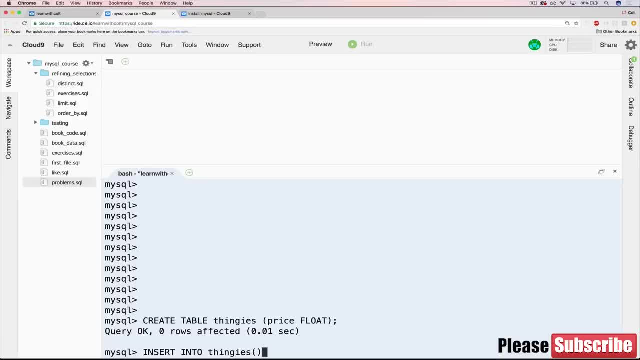 So then we'll do our insert into thingies and we'll do what we need to do: Price values, and let's start with a simple one. Let's do 88.45, and if we select that out of there, good, we get 88.45, but we'll run into problems. 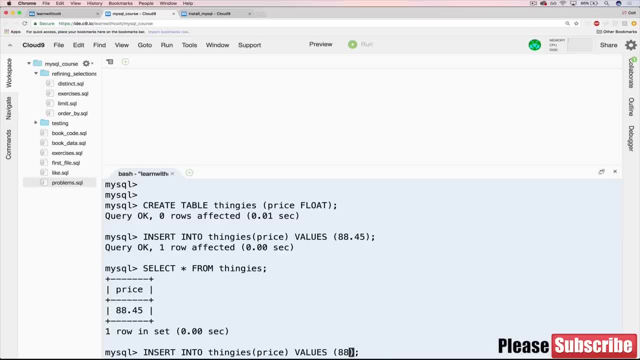 If we start making more complex, longer numbers. So let's do something like 8877.45 and that should still work. If we select it out, you can see it's unchanged. Remember, we're working with 456 characters here and if we go back to that table that I had says around seven issues. 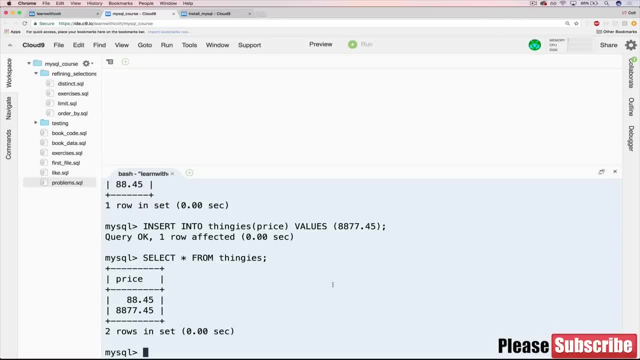 we run into precision problems. seven characters and run into precision problems. So if we do something a little longer, now 8877665544 and we hit enter, Notice how it got stored. So it doesn't just truncate, It doesn't chop things off. 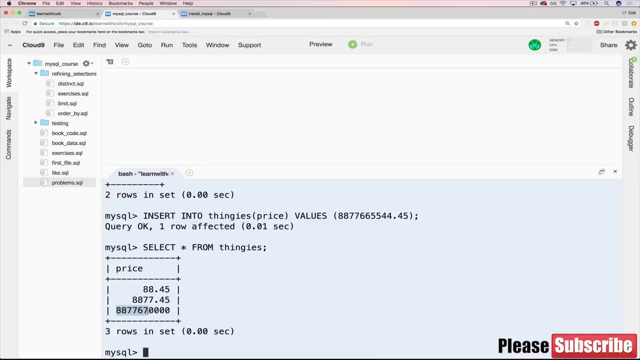 but it only stores the first seven digits and then it just puts these empty tens places- Well, not tens places, but it multiplies by 10 at zeros, essentially at the end. So we end up with this, which is very different than this. 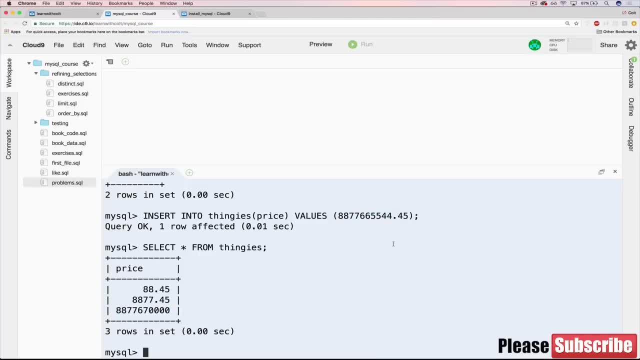 And if we instead had this as a double instead of a float, we would have that precision extended out to 15 characters. So it is significant and it makes a big impact, depending on what you're doing and what you need, Um, so that's why I recommend using decimal, where you can control exactly what you need and how long you need things to be. 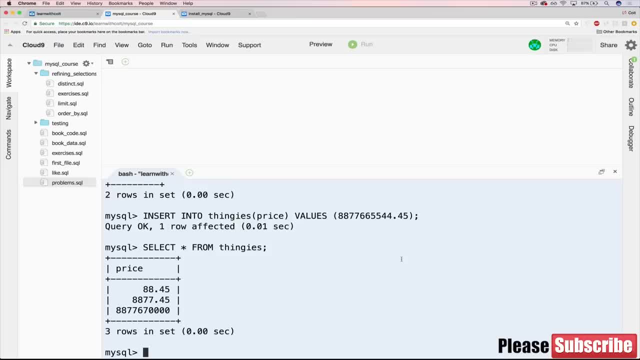 However, if you're working with gigantic numbers and you don't need to be that precise, you can use double or float, but typically my rule of thumb is, if you need to use one, use double rather than float, because you have you know. 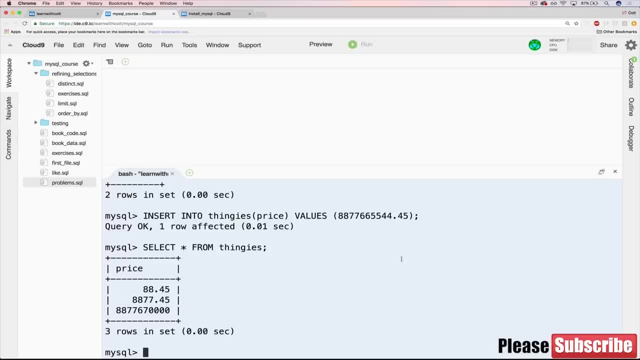 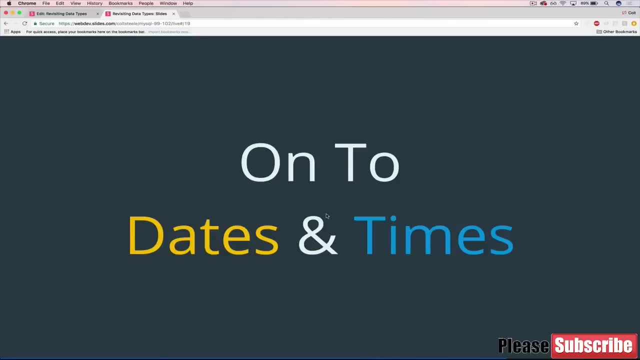 15 characters, 15 places of precision rather than seven, you get double the precision. Okay, All right. So we've made it through that war zone of string and number types. in particular, The number types are always a bit hairy, but we're moving on to something equally finicky: dates in times. 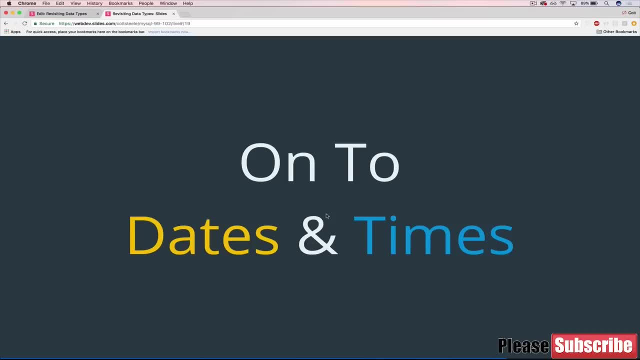 Often the bane of many programs programmers: existence, having to deal with time zones and synchronizing things across the world and daylight savings, And it's just a nightmare, We peers. Fortunately, my SQL makes it relatively simple for us. I'm going to show you how in just next couple of videos. 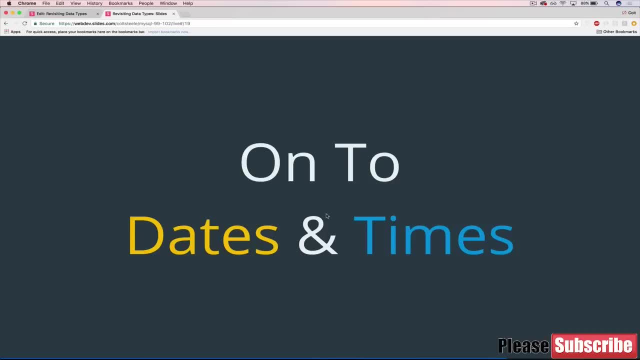 So this is going to be a series here, not just a single video, And in fact in this first video I'm just going to give you a quick overview of the three important data types that we'll take a look at. So the first one is called date. 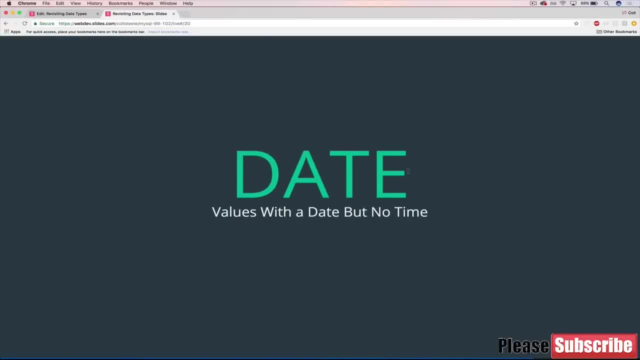 And what it does is it just stores A date without a time. So the format looks like this: year, year, year, year year dash month, month dash day, day, So 1999, dash 11, dash 25 or something. 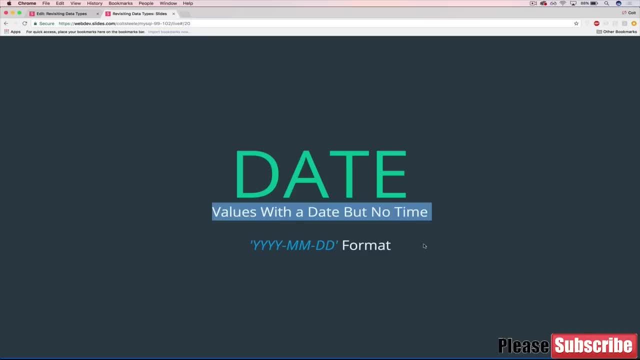 So, as it states here, that's that stores a date but no time. So there are instances where you may use this things like a birthday, If you're asking a user to- uh, you know, sign up and specify their birthday. 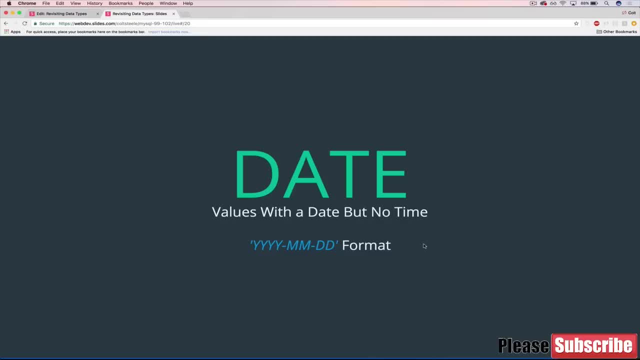 Most users don't know the time. Well, I don't know. I don't know the time I was born. I know a lot of people do, but it doesn't matter. At least for most websites. it doesn't matter what time someone was born. 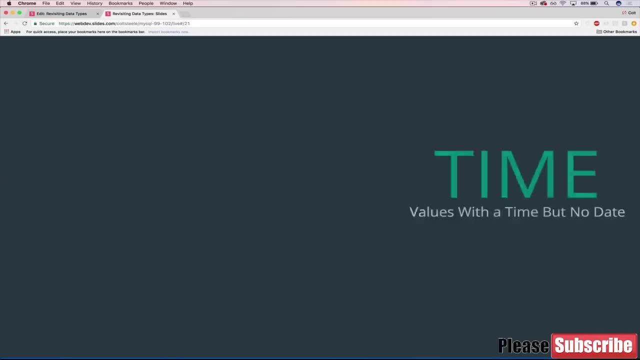 You just need that date. Another option is the opposite: The time. So time is another data type that stores values with a time but no date. So out of the three I'm going to show you, this is the one I use the least by far. 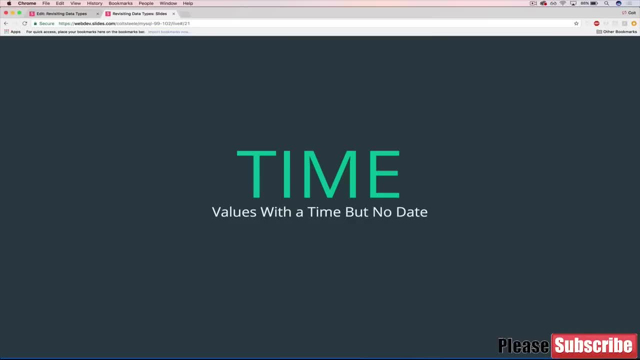 because there's not many things that you just need to store The time. maybe if you're- I don't know if you're- working with uh, reminders maybe like are working- I'm at a loss really- but basically you store times and the syntax. 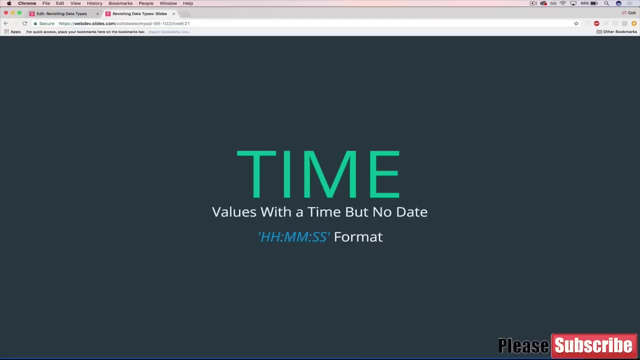 the format is our hour, dash or, excuse me, colon, minute, minute, colon, second, second. And the final data type, and the one that I use by far the most out of all of them, is date Time. Not very creative, I know. 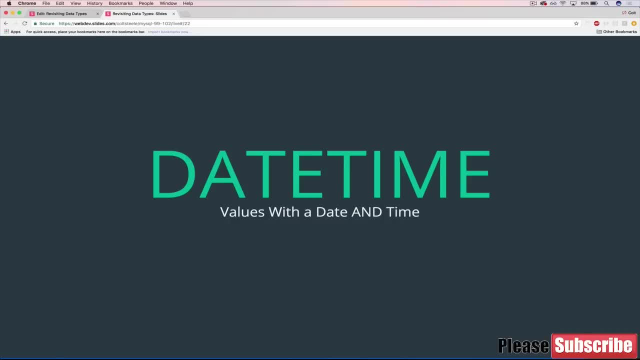 it's just date plus time- does what it sounds like- which I also realize I'm saying way too often in this course- but it stores values with a date and a time And this is pretty useful. You get both Um and, like I said, 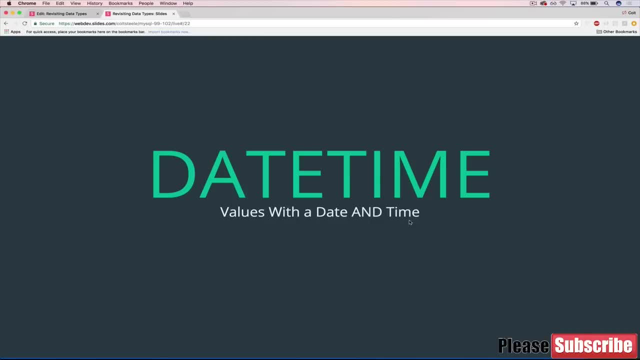 this is what I use the most. So when you're doing things like I don't know when a user signed up for your site or when something was last updated, uh, you know when a profile picture was last updated or when somebody commented on. 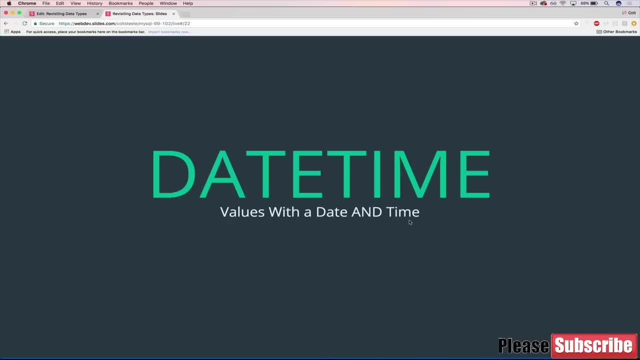 a Facebook post, those are all stored with date times, because just having the time on its own isn't that useful, So let's go with this Facebook example. You know, if I comment on someone's post, um, Facebook doesn't just store the time that I commented. 10,. 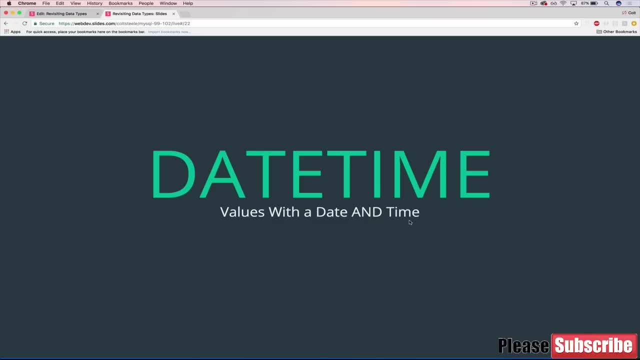 39 PM, let's say, because it's just not that useful to them. You know, I think, what Facebook does. it displays things like: uh, how many days ago, or hours or minutes ago, or something you know, I commented. 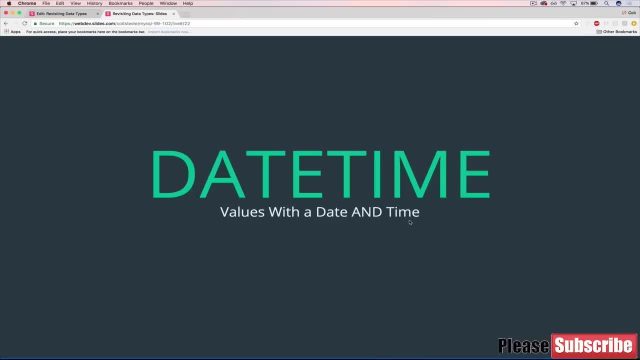 it will say, like Colt commented three seconds ago, 20 minutes ago, two days ago, last month, and it needs more than just a time to figure that out right, It needs a time and the day. So date time very. 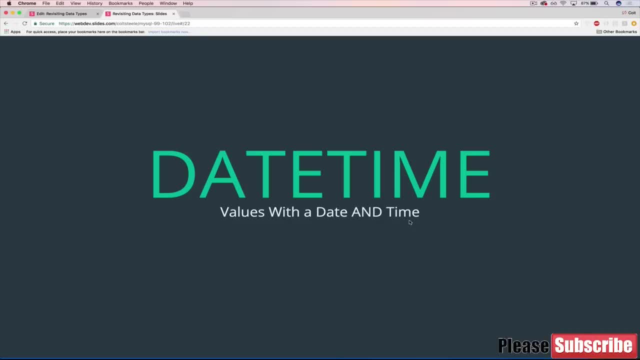 very useful and used all the time in applications, And a really common use case, uh, in programming in general, is when you have a column or, let's say, a row in a database, in a table, and it's created. you often want to just store the date and time it. 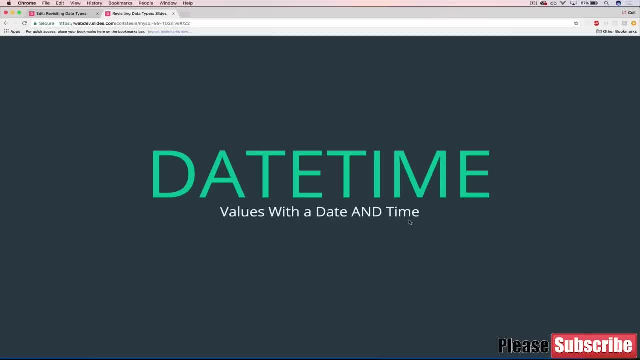 was created so that you can then go and sort things based off of how new they are and how old they are. So very easy You know if you're working on comments, for example, going back to Facebook. Facebook comments are displayed in the order that they were. 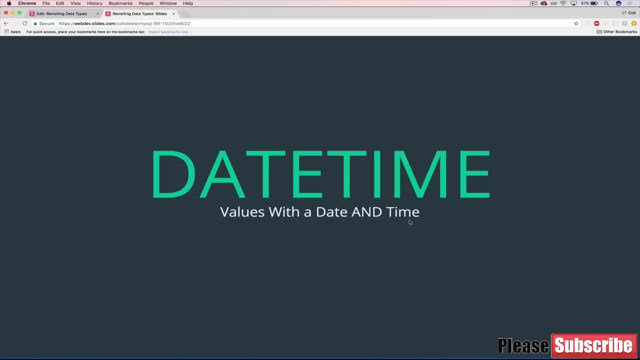 written and posted, So you need to store that created at time. So that's where date times come in And the format is also what you probably expect: year, year, year, year dash month. month, dash day, day, which is the date part. 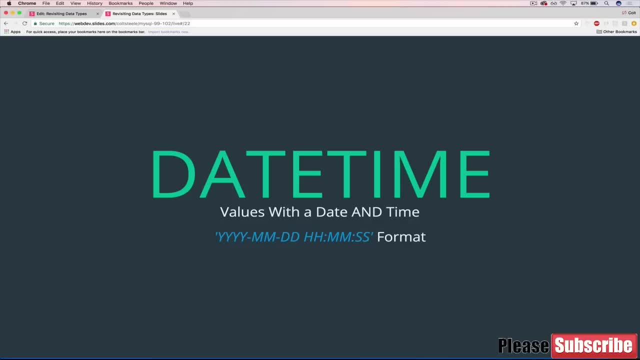 And then a space, hour, hour, colon, minute, minute, colon, second second, which is the time component. Okay, So we talked about those three. We didn't see them in action, but we saw that they exist: date and time and date. 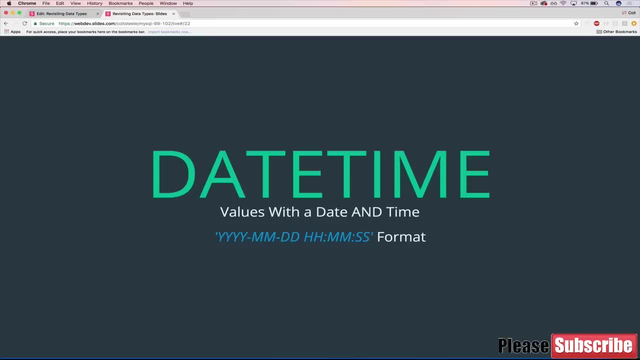 time And again, I use date time. The most we'll be using it, the most it's the most versatile and the most useful. So now that you've seen the three data types we're talking about here around dates, which are date time and date time. 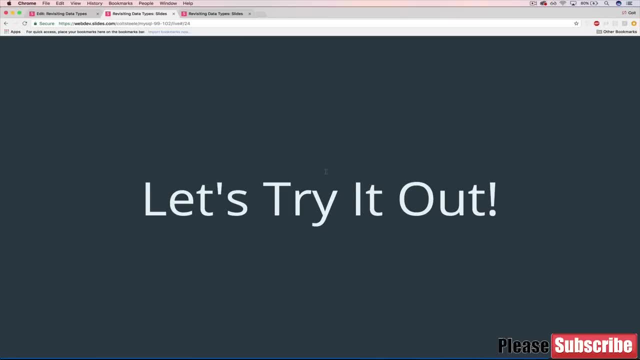 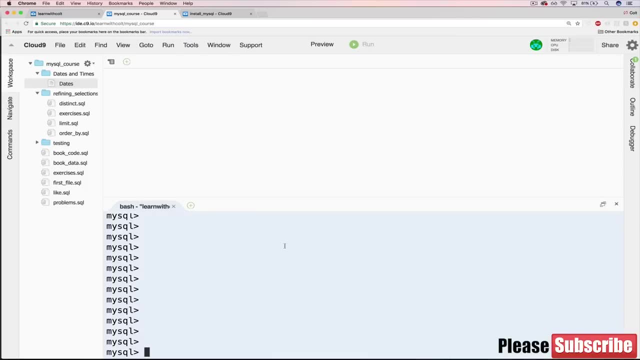 let's hop over to cloud nine and just try them out briefly. So what I'm going to do is actually make a new table, And in this one table I'm going to use all three types to three different columns, of course. 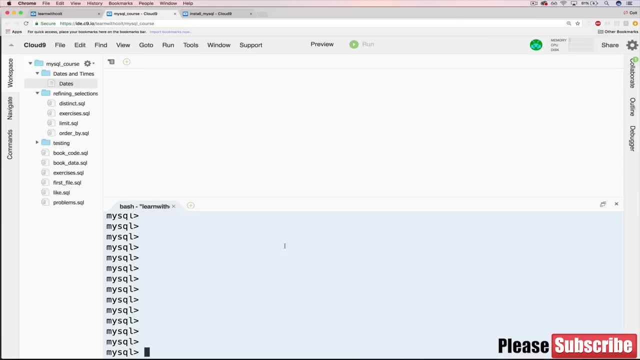 so that we can compare and contrast how they work And you'll see that they're pretty similar, honestly, which is why I didn't want to make three separate videos, because it would be pretty boring, It'd be a lot of repetition. 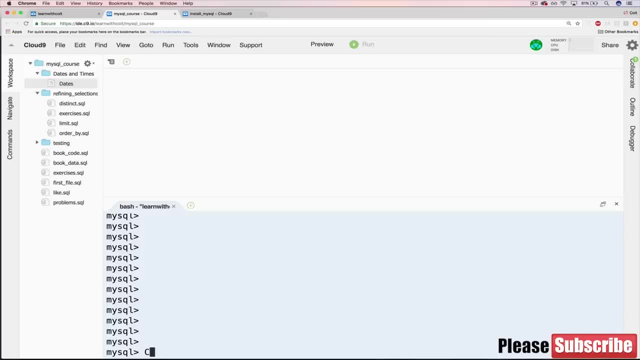 So let's go ahead and do this. Now we're going to make a table called people And in people we will have, we're going to work with a- well, we'll start with name, which will just be a VAR char. 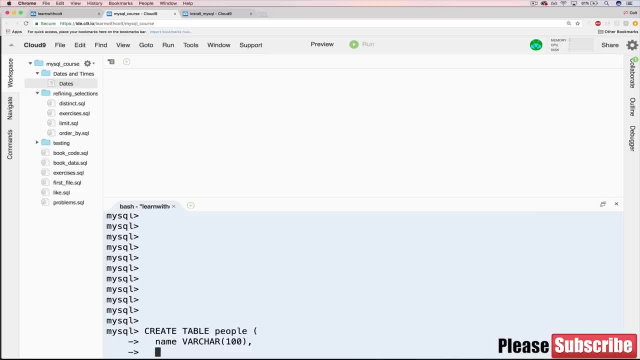 So somebody's name. then we're also going to have birth day as a date, birthday as a time and birthday as a date time. Of course we can't just call it birthday three times, So we'll start with: birth date is a date. 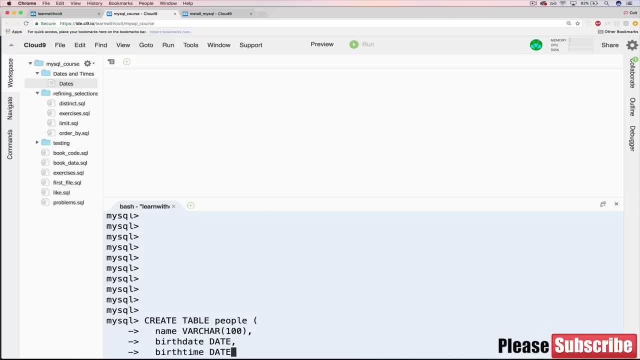 Then we'll have: birth time Is a time. finally, birth date Time is kind of annoying. Let's just do D: T is a date time, just like that. Okay, So we have that table now with name, birth date, birth time and birth D T. 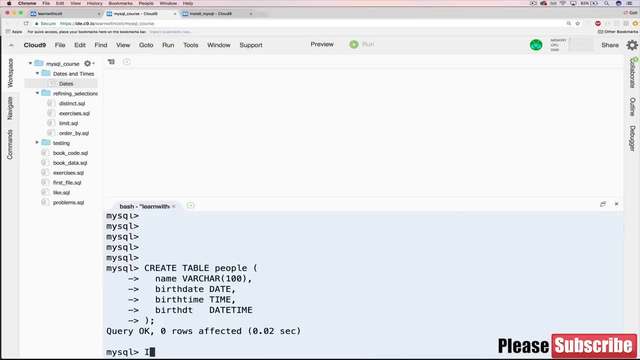 So we're not going to spend a lot of time adding data in, but let's insert at least two. So let's do, Let's do an insert into people and we'll start with name, birth date, birth time, birth D T. 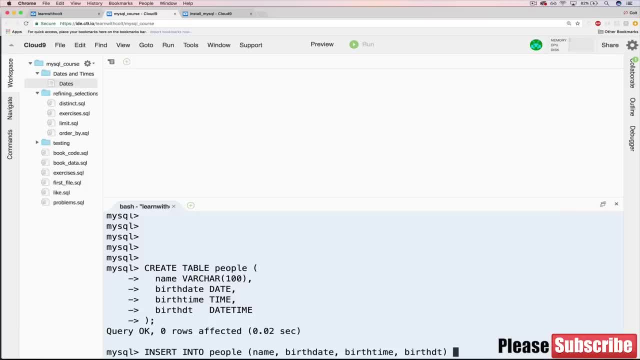 Okay, Just like that, And then on a new line. this is going to be the worst part, So let's make up a date. Well, a name first of all- let's say Padma- And then the birth date. 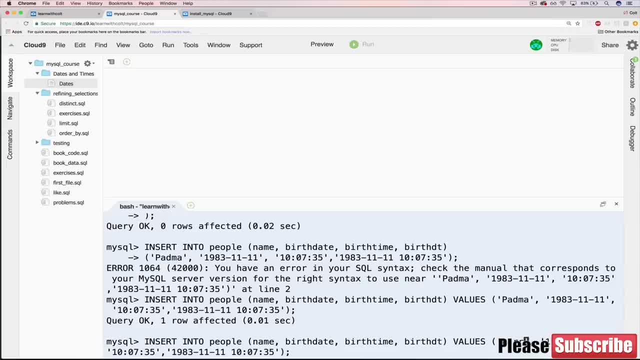 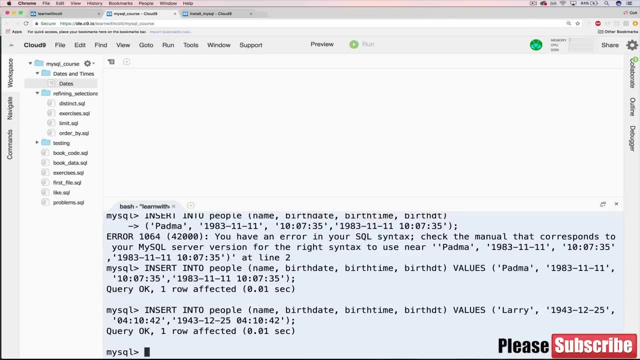 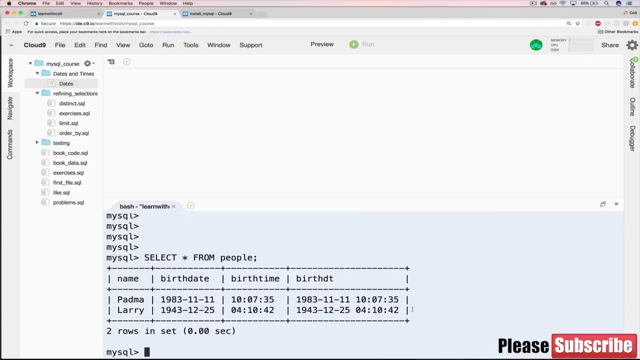 Remember we need that year, year, year dash, month, month dash day, day format. So we will do 1983 dash, Let's do 1111.. So that's the birth date. Then the birth time needs to follow hours. 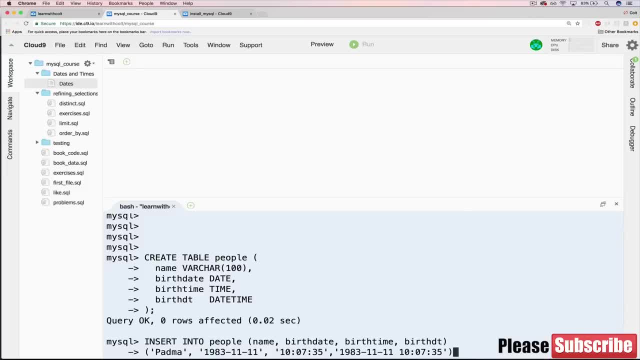 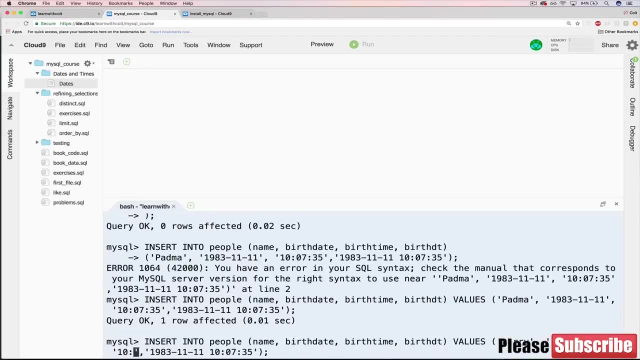 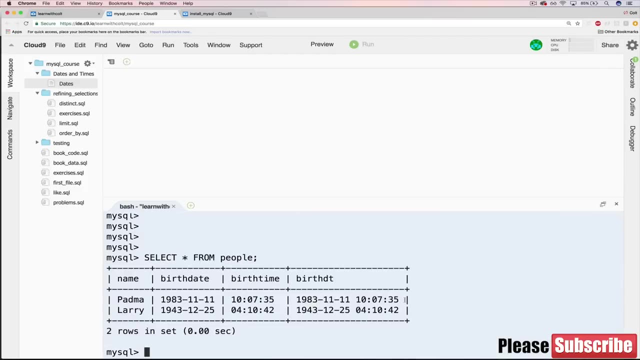 minutes second. well, our our colon minute minute, colon, second second. So let's say 10,, oh seven, oops 35. And then, if we want to be accurate for the date time, we'd basically combine these two. 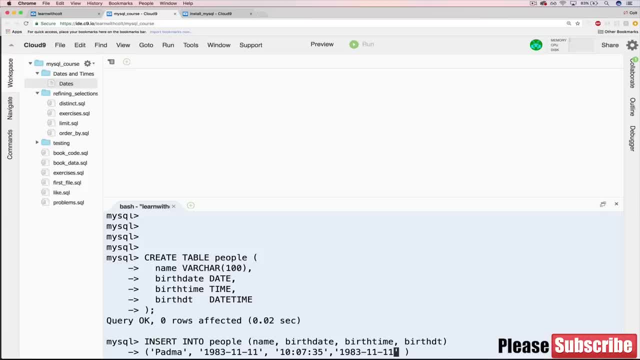 So we would have 1983 dash 11, dash 11 space in the same time. Okay, So that's kind of annoying to type. Uh, you're usually not doing things like this, to be honest, but let's just make sure we don't have any typos. 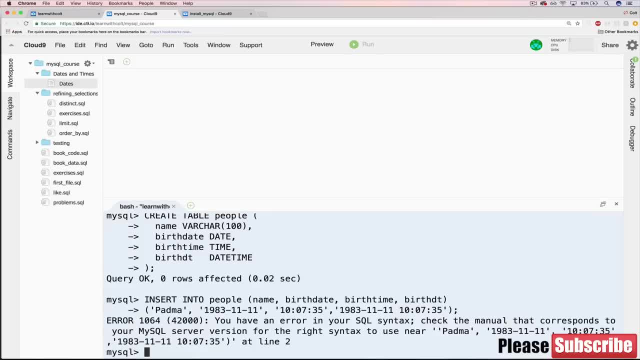 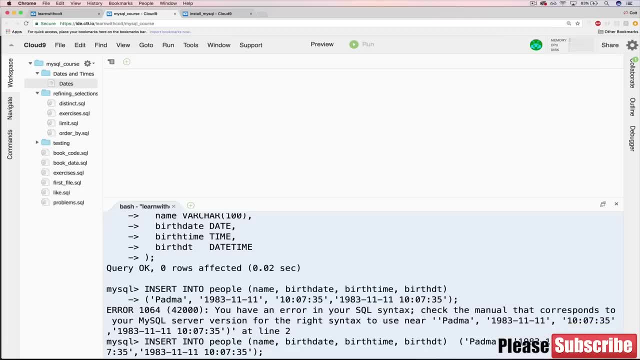 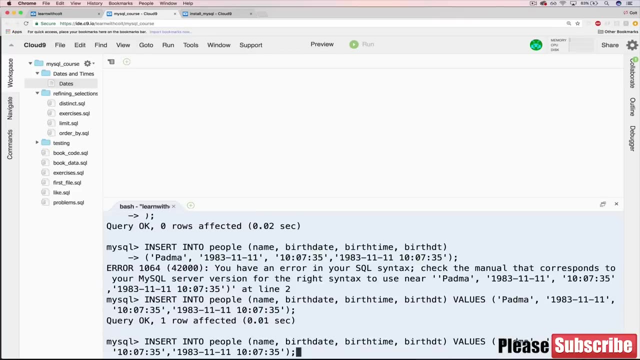 I'm not missing any quotes. We'll soon see. Oh boy, We do have a problem, And this is a silly one: We're missing the values keyword. Hopefully you caught that before me, Okay, So I'm just going to recall that and just change some information. 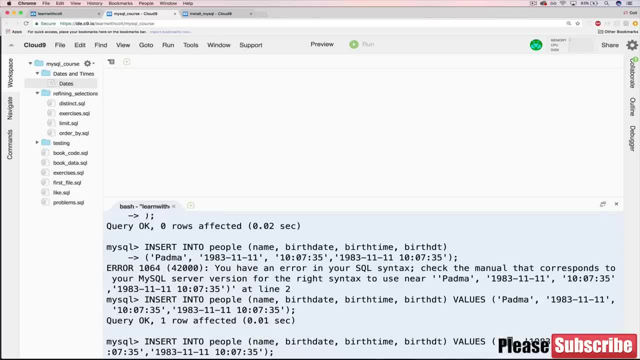 So we have two people in there, So we had Pat. uh, let's put um Larry, who was born in 1943, and on December 25th, on Christmas, at um, let's do four: 10, 42.. 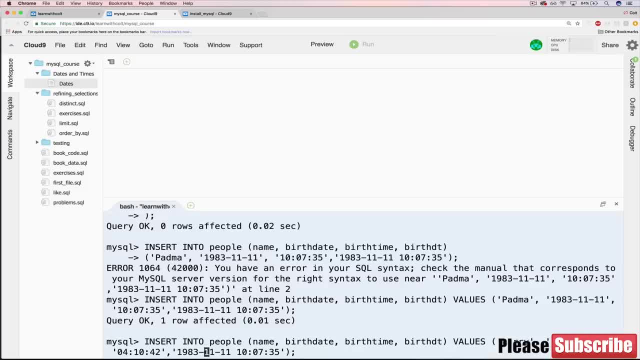 And then we'll just copy this so we don't have to retype that whole thing. I apologize, It was a little bit painful to sit through. We're not doing much, but we need some data to work with, Okay, So that should be sufficient. 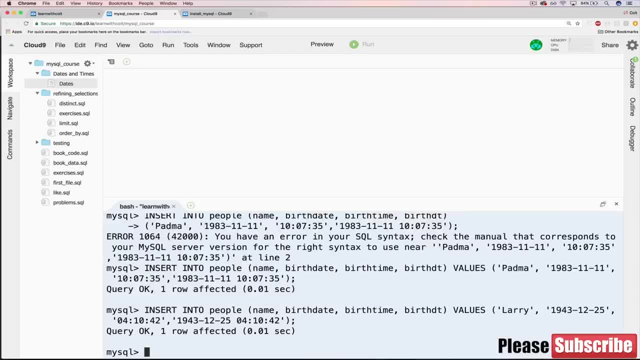 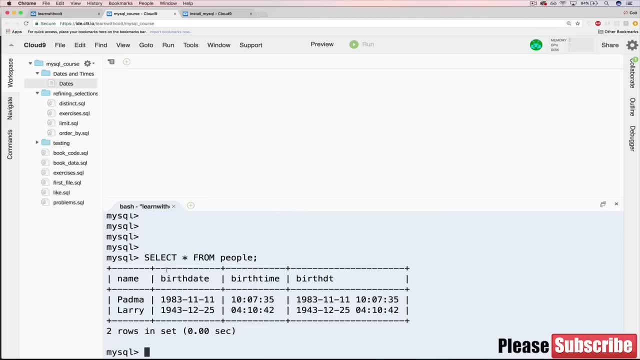 Now just make sure that matches up, All right. So now we do a select star from people. We have two people in there and then we're storing birth day information three different ways, although they're not equivalent, of course, because we have just the date. 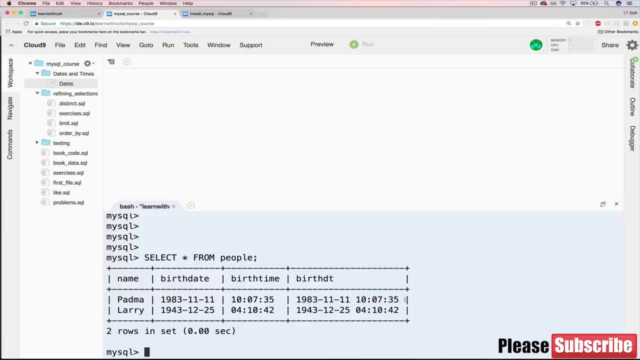 just the time, and then the date and time together. So now that we have this data in there, we're going to focus for a couple of videos- pretty short videos- on how we can work with this data. There are some functions that come with my SQL. 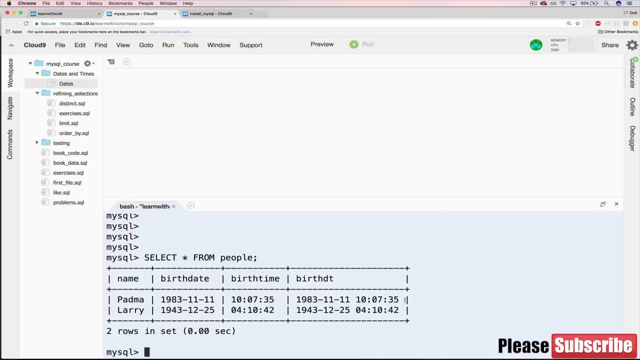 which- and we've seen a bunch of them, but there's some that work with dates and date, times and times and we're going to focus on Those to do things like format our data nicely. So how do we format dates? How do we get the day of the week based when? 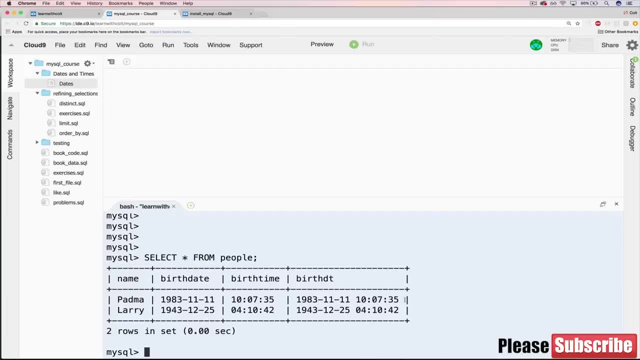 based off of someone's day- they were born, things like that. And how do we print out a nice version? This is a little bit ugly. And then also, how do we do math with dates? Now, we're not going to do any heavy duty math. 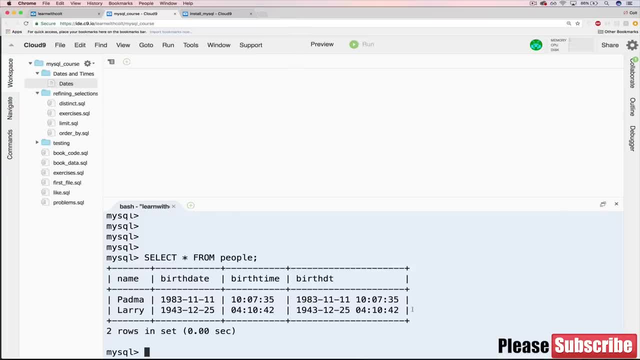 but things like calculating how many years it's been from 1943 to now or how many days since Padma was born, Those sorts of things, And we'll be able to do that now because we have this data in here. So thanks for sitting through that. 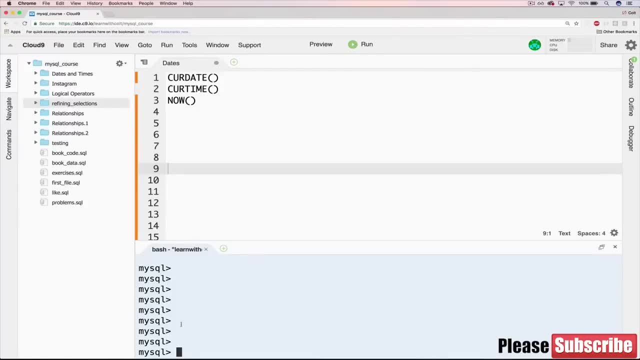 I know it's probably a bit painful. Hey there, So I have a small confession to make at the beginning of this video. This is not my first time recording this. I recorded this about a month ago, along with all the other videos in this section, and something happened. 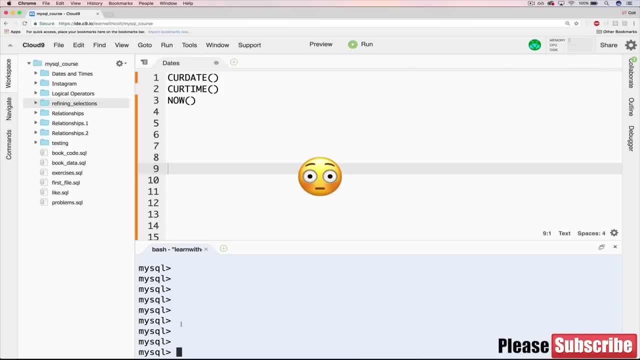 I didn't save it correctly. I maybe accidentally deleted it. My cat stepped on the keyboard. I have no idea, but the original video here is gone And normally that wouldn't be a problem. I it's happened before or I just rerecord a section cause I'm not happy with it. 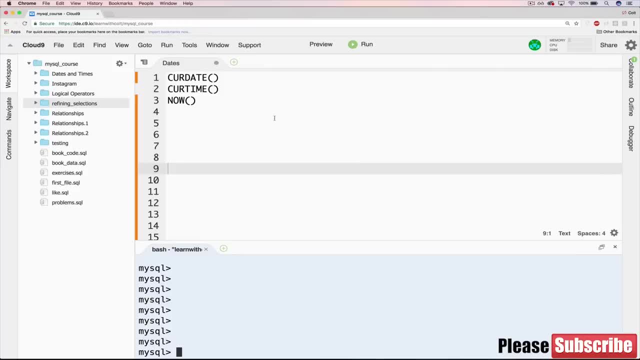 You know, that's not too bad, That's easy to do. But since this has to do with dates and in particular it has to do with these three date functions that I'm going to show you. Basically, they give us the current date. 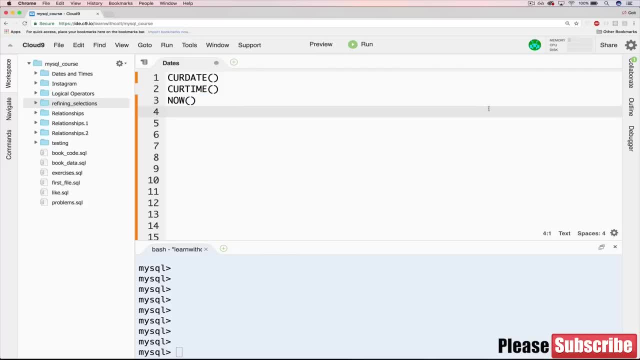 the current time and the current date time. You'll see in the videos following this one that the code that I ran when I was recording it the first time resulted in different dates and different times than what you'll see right now. So it's not a big deal at all. 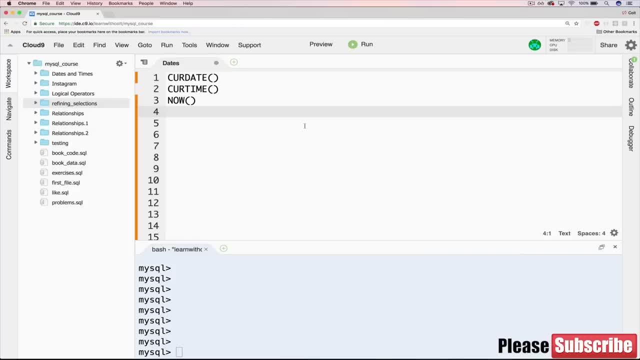 It's just evidence that I recorded them on different times, but I wanted to just let you know what to expect. Okay, So in the last video we inserted these two, or we manually created or basically wrote out the dates: the time and the date time. 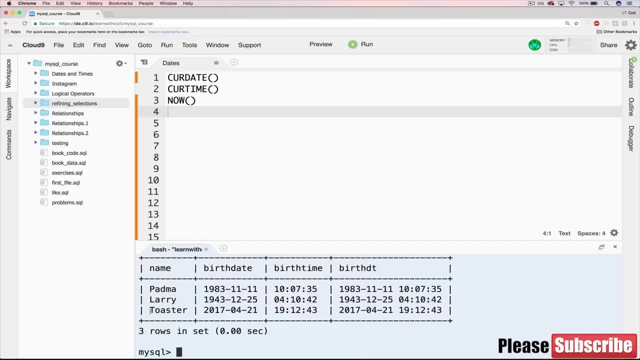 Um, and then in the initial recorded version of this video, this is the new person that I inserted and this uh: birth date, birth time and birth date time. We're all done using these three functions here that give the current date time. 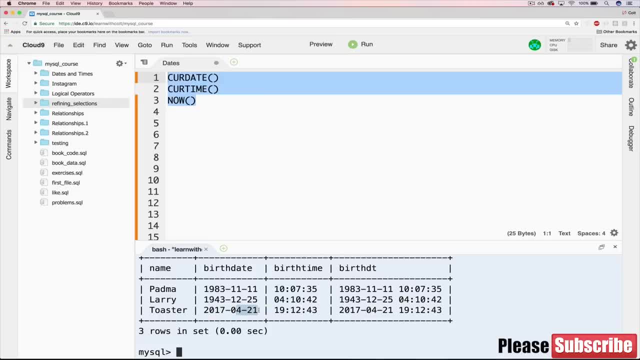 The current birth or the current date. So at the time it was April 21st and the time was seven 12 and this was the date time, And so I used these to generate this. So in the next video you will see this person with toaster birth date. 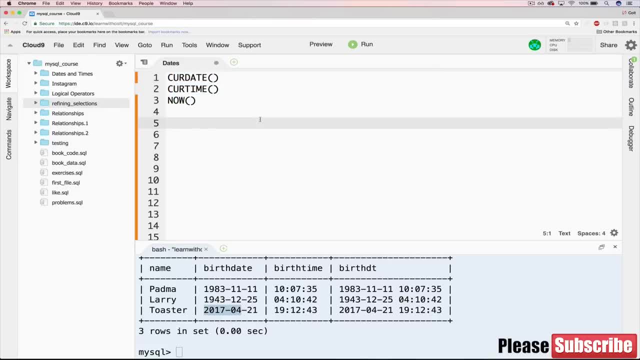 April 21st and so on, But in this video, where I'm actually showing you the creation, I'm having to rerecord it, So there's just a small discrepancy. other than that, everything else will be the same. So let me show you these three methods here. 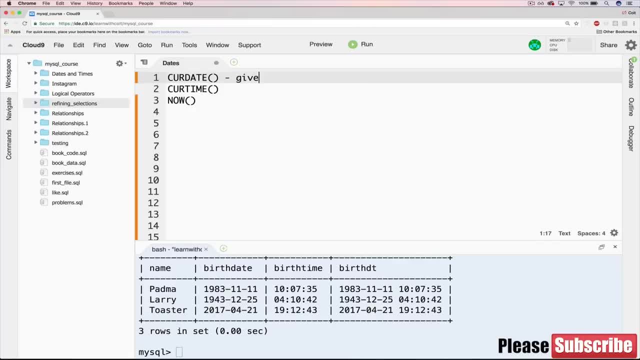 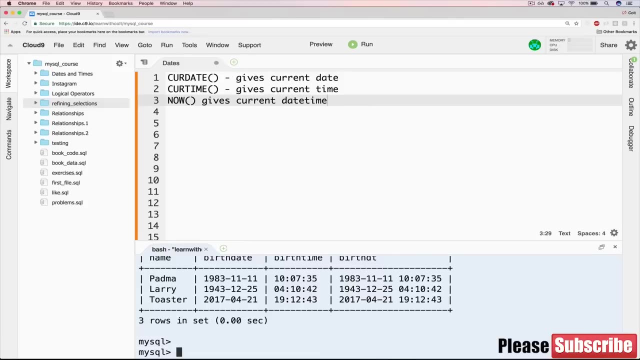 They're really useful, simple things. but Kerr date gives current date. As I said, Kerr time gives the current time and then now gives current date time. So let's try one of them just on their own. If you did something like select Kerr date. 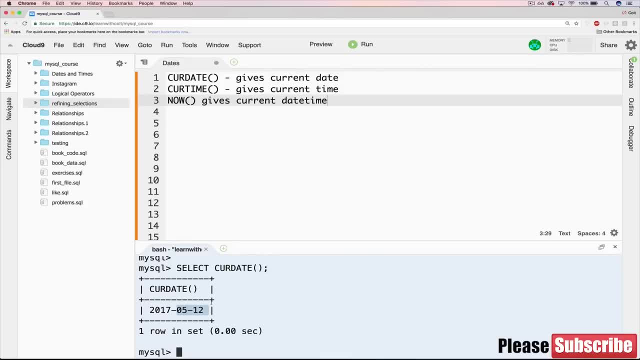 you'll see that I'm actually recording this on five, 12, May 12th, So not quite a month later, but a couple of weeks later. So if we do the same thing with Kerr time, we get the time, and then if we do now, we get. 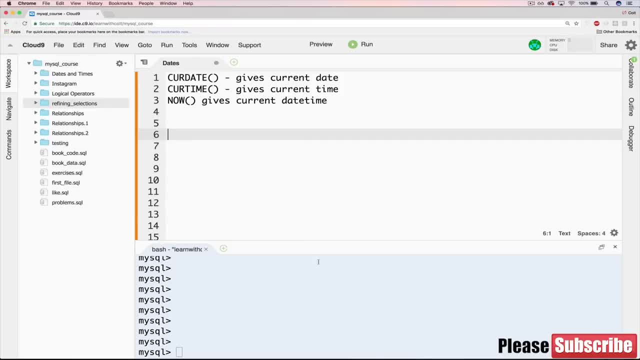 the date time. So using them on their own is not useful really, just to select the current time. It's much easier just to look at your watch. but they become useful when we use them in conjunction with insert statements, So things like when we're inserting a new user and we want 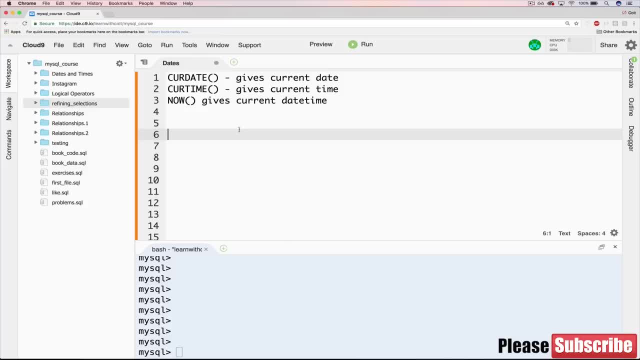 to save the time that the user was inserted, what we can do is basically write, Okay, Insert into and we'll do people, Let's do our select star from people. Okay, So we'll do insert into people birth date, birth time and birth date time. 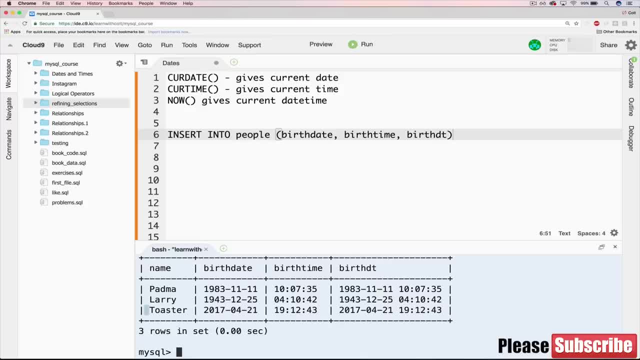 And so the I think the hypothetical story I gave was that toaster was my son, my first son, and he was born exactly at the moment when I hit enter. So we'll do the same thing here, Inserting into people birth date. 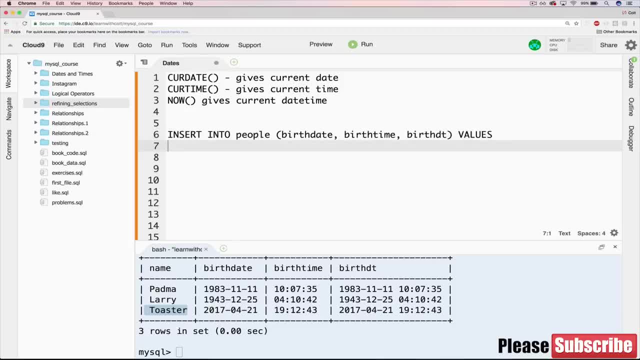 birth time. birth date: date time. This will be my new son, and this one's name is: let me actually add name as well. Oh boy, I'm really bad at naming things. You can tell I named my cat blue. 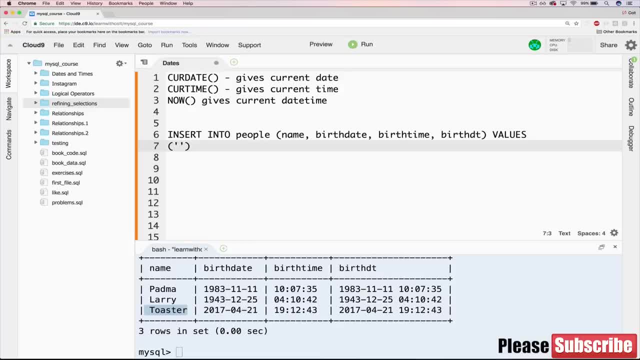 which is a blue steel, by the way, if you didn't catch that. Okay, So I'll name him microwave. And then, rather than writing out the giant date here, what I'll do instead is for the birth date, I just say current date. 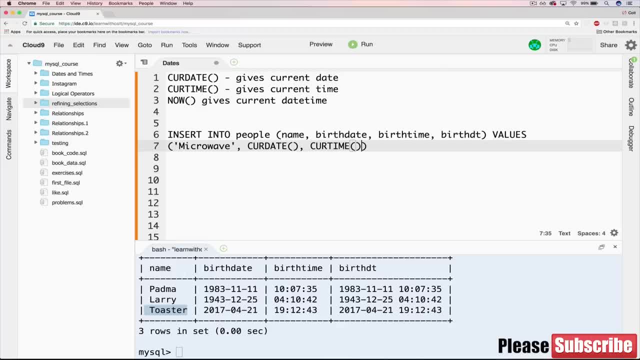 And then for the birth time I'll just use current time, And then for birth date time I use now, And out of all of these, I end up using now the most often because, as I've mentioned before, we use date times a lot. 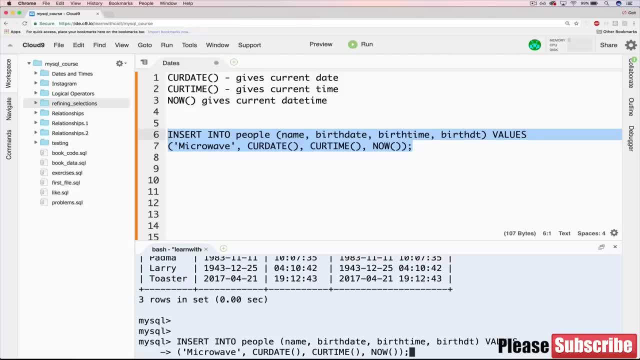 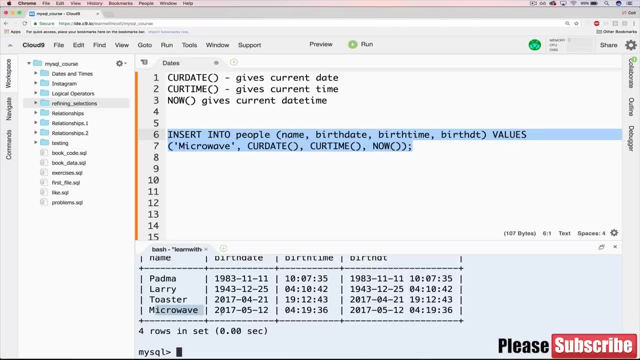 Okay, So if we just run this right now and insert that and now we do our select star from people, you can see that microwave now has the date, the time and the date time that reflect exactly when I inserted this just a couple of seconds ago. 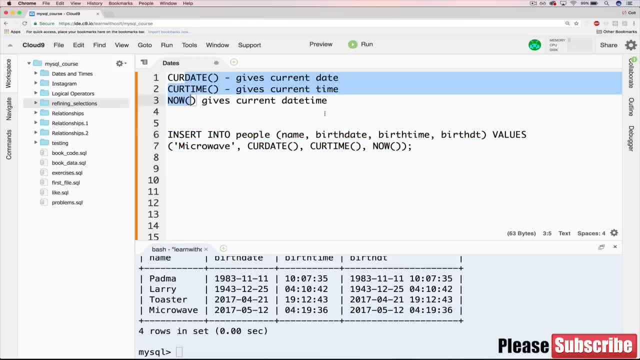 And that's pretty much all there is to these, these three nice little functions. Another way that we use them, by the way, it's not just to insert data with current dates and times and so on, but also to compare data to the current time. 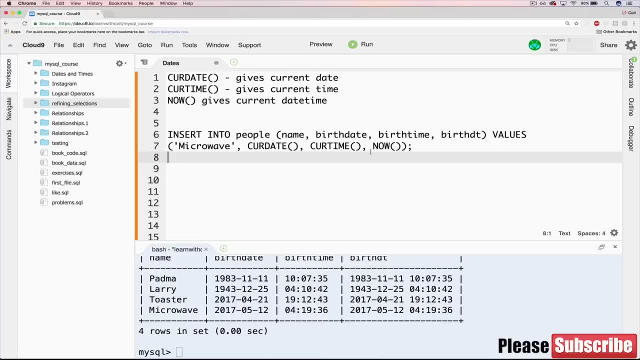 So I'll show you how to do some basic date math. We'll be able to figure out you know how long ago something was compared to now, And so we need to be able to refer to now. or you want to figure out how many dates. 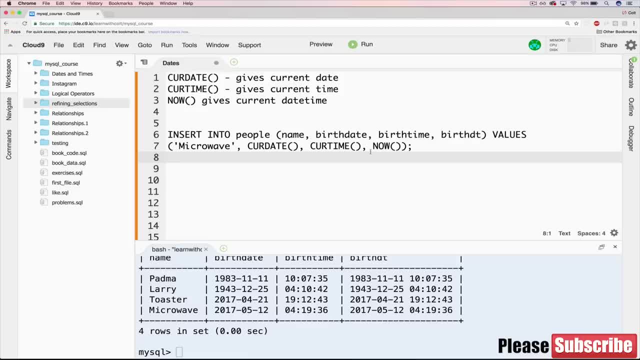 you know how many days somebody was born ago compared to the current date. So we need that current date in order to help out with that Math. Okay, So the last thing I'll do here, just for continuity sake, is delete microwave so that we have toaster Larry and Padma. 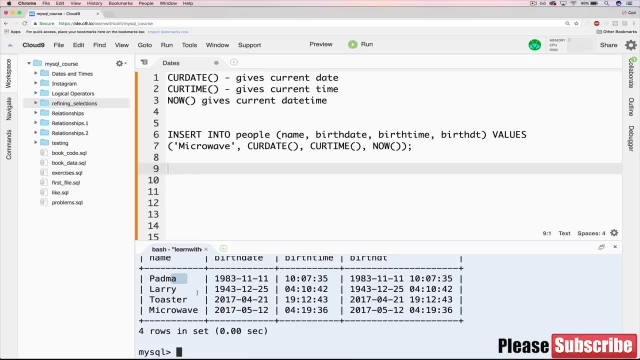 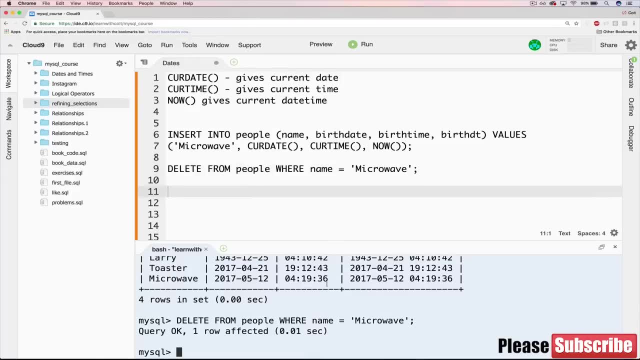 which is what I had in the original recording, so that the next video here- hopefully it will be relatively seamless. So I'm getting rid of my son. I'm sorry, microwave, I failed you. Okay, Now he's gone and we're back to these three. 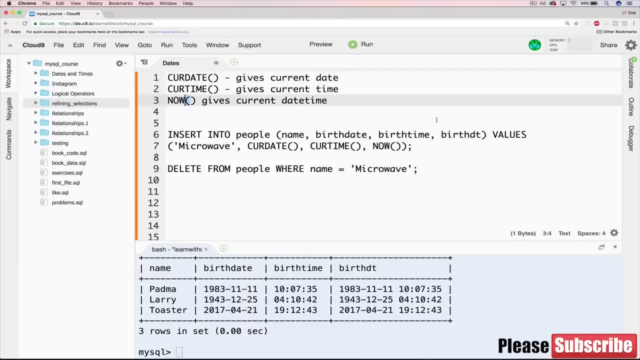 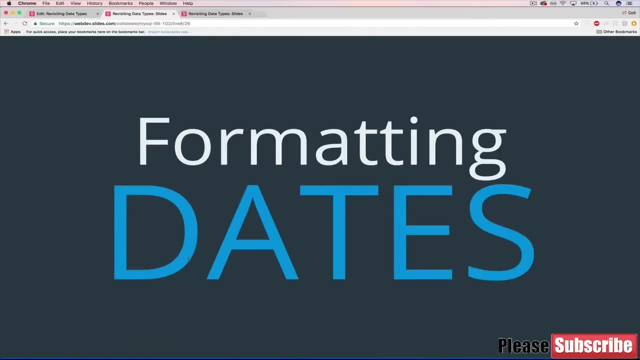 All right. So that's current date, current time and now All right, Welcome back. So in this video, we're continuing with not the most exciting topic potentially, I know, but an important one nonetheless. So we're talking about formatting days right now. 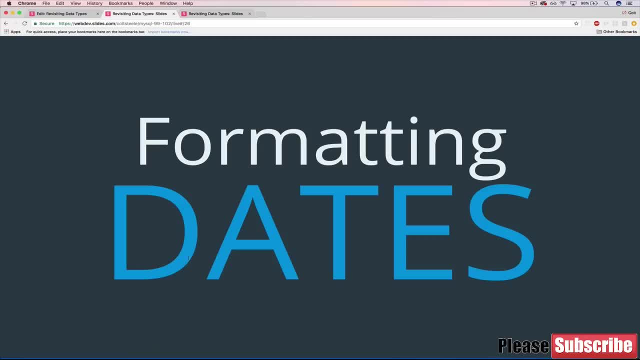 We have dates times, date times- all stored in a somewhat clunky, condensed but difficult to read, at least for human difficult to read format, just not very nice. So how can we extract things out of, let's say, a date time? How can I convert that so that it says something like April 21st? 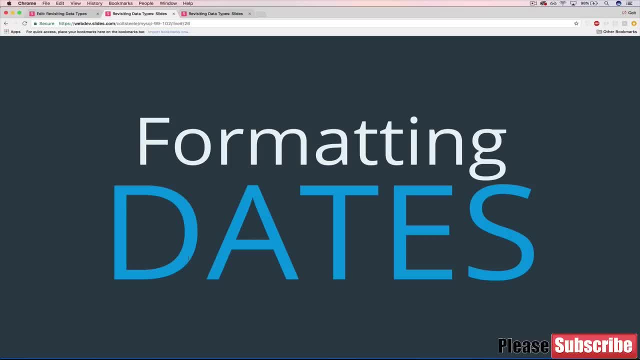 like the full month, month name followed by a space- 21st to one, S, T, and then the full year, rather than, you know, 2017. dash Oh four, dash two, two. So we're going to do that. First thing I want to show you, though. 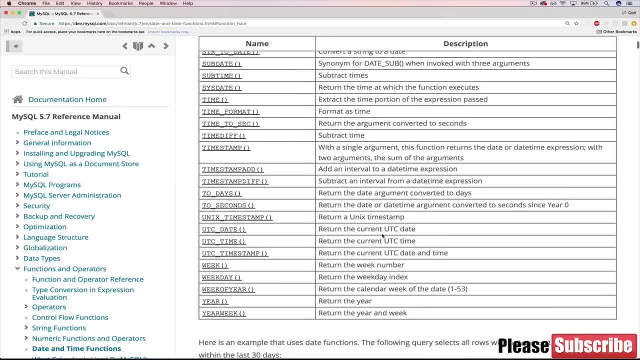 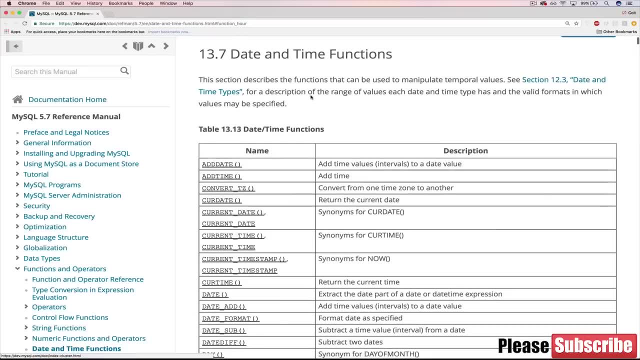 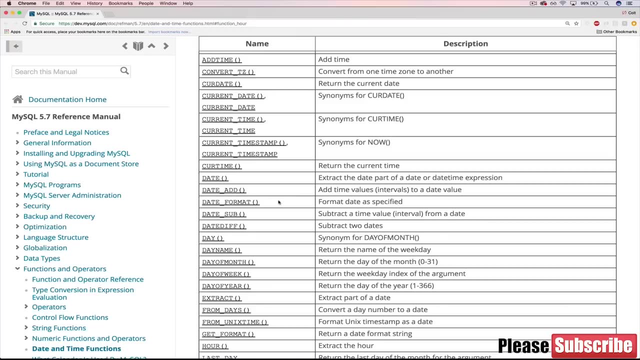 is that in the documentation there was a pretty massive list of date and time functions and I will be honest with you. Uh, most of these I never use and you likely will never use. That won't stop me from showing some of them to you and I'm going to try and highlight which ones are most important. and the first few I'm going to show you I don't actually think are that important, but they're nice to know that they exist and they're a set of these one off little functions. 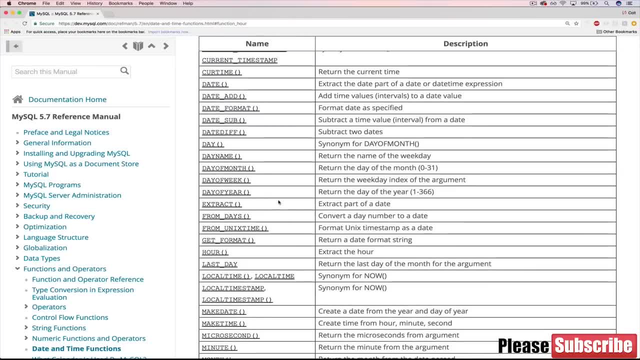 I'm not sure even what to call them, but basically there's a group of them, at least in my mind. I group them together, things that will extract an individual piece of information, like day or day name, or day of month, day of week, day of year. 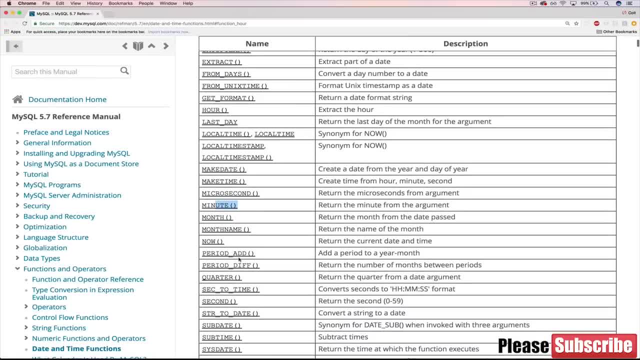 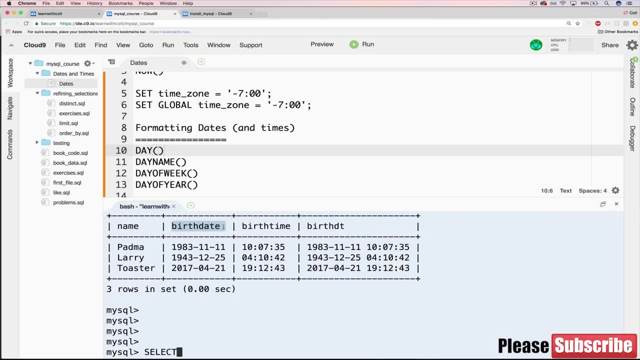 hour, month minute. So let me show you what I mean. So I'm going to hop over to cloud nine and we have a select star. Let's only work with birth date for now. So we'll do select name, birth date. 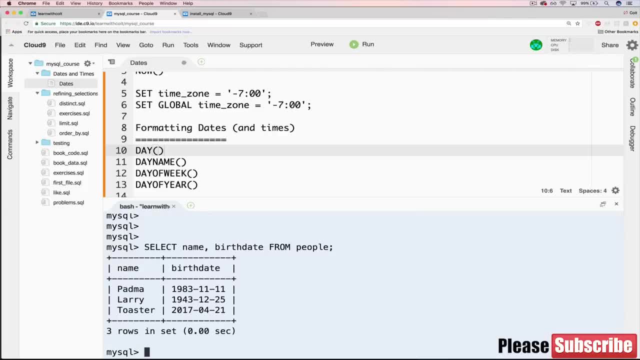 from people. Okay, so instead of displaying the date here or the entire date, what I can do is I can select date and what I can do is use some of those things that we talked about. whatever that group is, Let's try day. 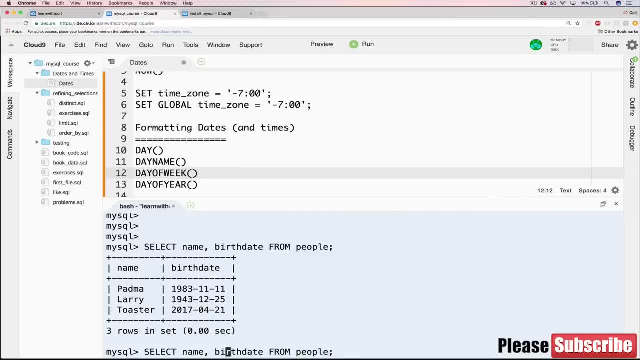 You'll see what it does. So, rather than birth date, I'll select day of birth date, and all that it does is extract the day. So if we compare, actually what might be better is if I keep birth date and I just add in an extra column with day. 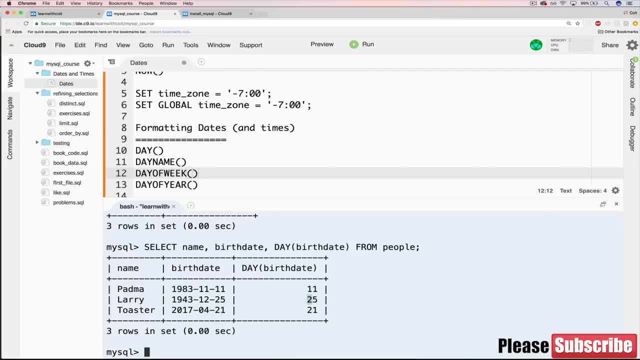 So it's extracting the day 11,, 25, and 21.. So there's other things we can do. Let's just go with this list. I have up here day name And this is a bit more useful. There are times when you want to do this. 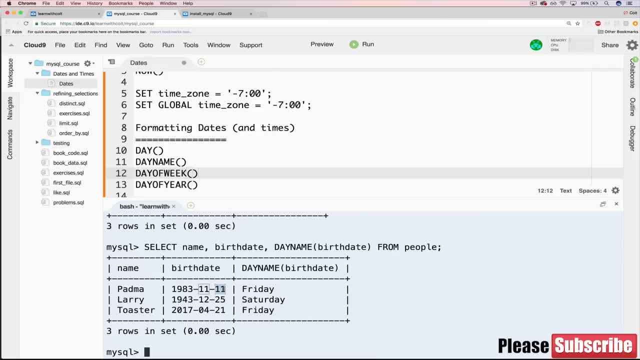 As you can see, we're extracting that. So turns out, this is a Friday. This is a Saturday. This is another Friday. I know some people can figure this out mentally. There's a whole trick to doing it. I'm not one of those people. 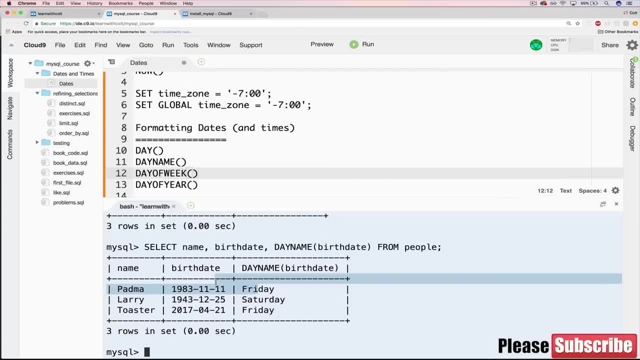 So we just have to trust it That this is indeed a Friday. Moving right along, we can try day of week. And you might wonder: how is that different? Well, it gives you a number. So a Friday is a six, Saturday is a seven. 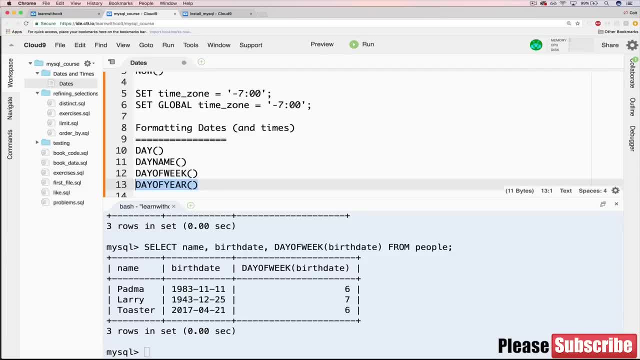 Sunday is a one, And so on. Then we also have day of year, And that will tell us, starting from the beginning of the year, how many days was it until? Oh boy, I messed up the parentheses. Here we go. 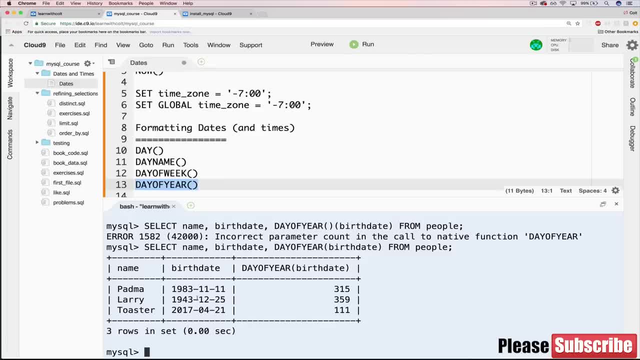 Until that date. So for something, on Christmas of 1943, it was the 359th day of the year. Oh my god, Blue, come on Blue. And this, of course, takes into account things like leap years, So important to know. 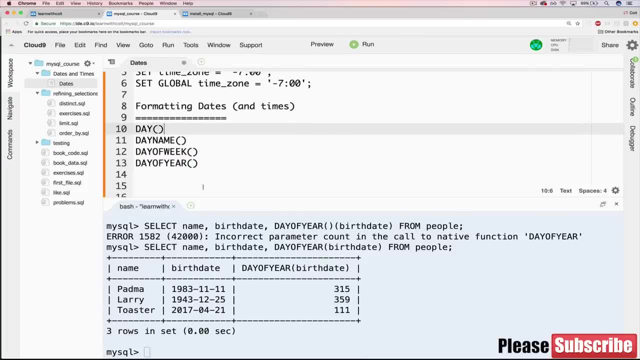 With that said, these also apply to date times. So if you tried to do it on time, if we start right there instead of doing birth date, and you tried to do birth time, well, there's going to be an immediate problem. 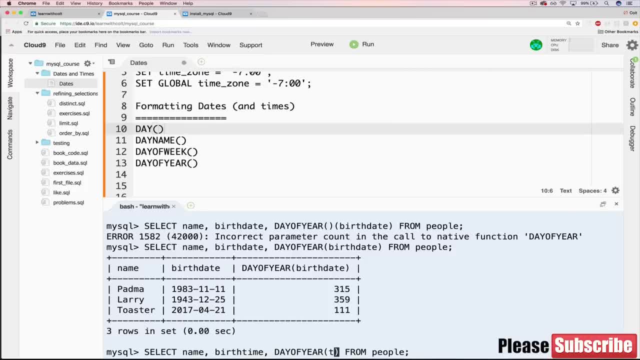 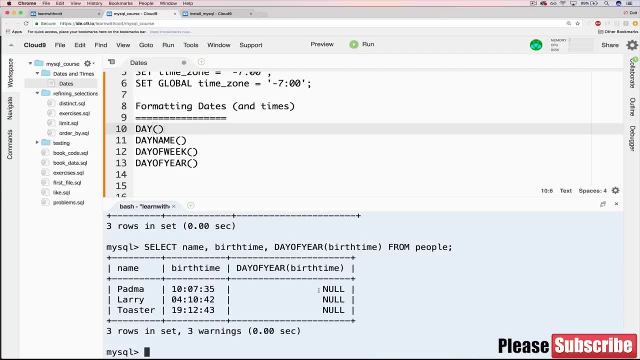 which is we're not storing day of the year or day information at all. But just to show you, we don't get an error right, We get warnings but we don't get something that breaks everything. We just get null. It doesn't work. 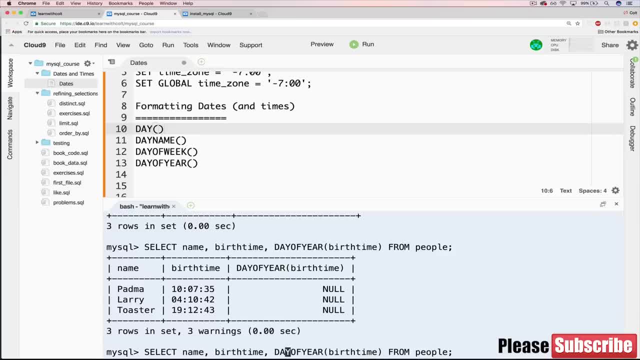 But we can do it on a date time And that's what, like I said, I use most of the time. So if we do birth DT instead, you can see that it's giving us the correct numbers here: 359,, 111, and so on. 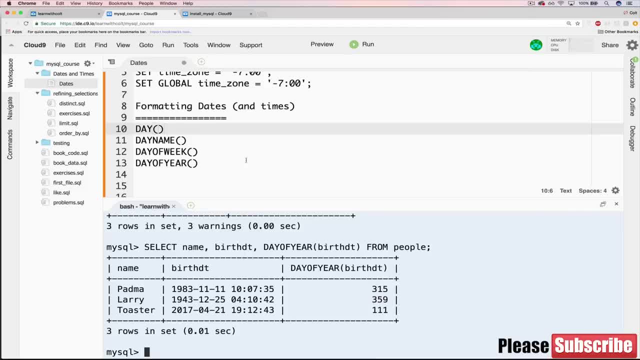 So we can use all of the ones we've seen, Day, day name. But there are other things, too briefly, that work for date and date time, So things like month. So that tells us the month. What else is there? 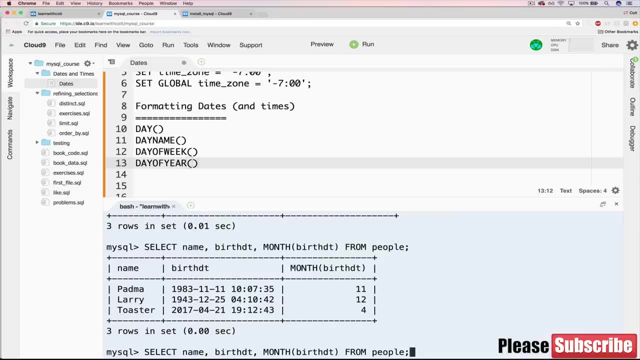 I think there's a month name, Yep. So if you want the full name of the month, there we go. And then, lastly, when we're working with the time, so if we go and change this to birth time, there are a few methods that apply here. 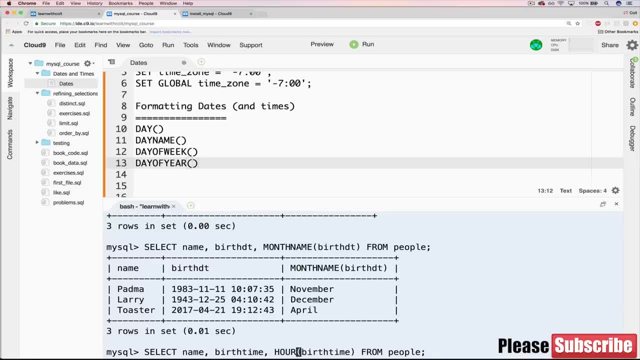 We can do things like hour if we want to extract the hour or minute. Now I don't end up using time on its own that often, so I don't really end up using these minute or hour or second on their own ever really. 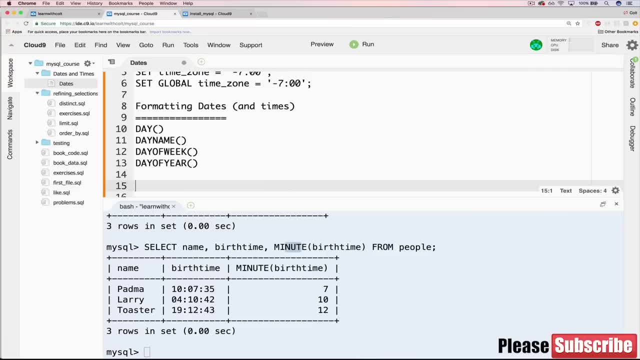 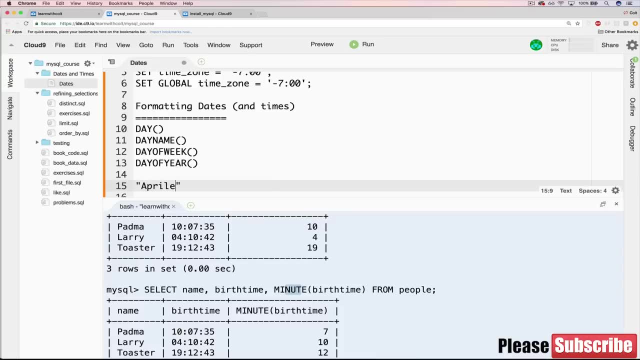 So that's part one of formatting dates. Imagine if you wanted to do something like this Instead of just printing out you know the day or something we wanted to say- April 21st 2017, at I don't know. 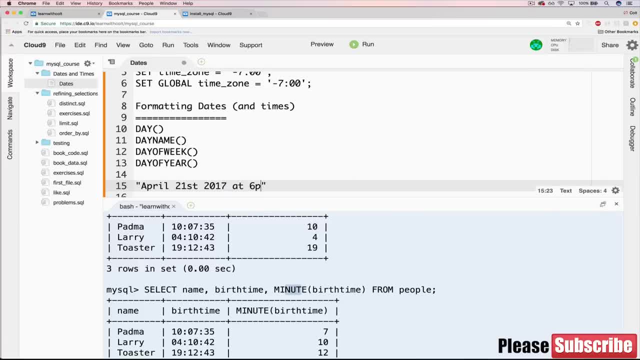 6 pm maybe, Or we don't even need that. Let's just say April 21st 2017.. So how would we take this date- that would be 2017-04-21, and convert it to this? 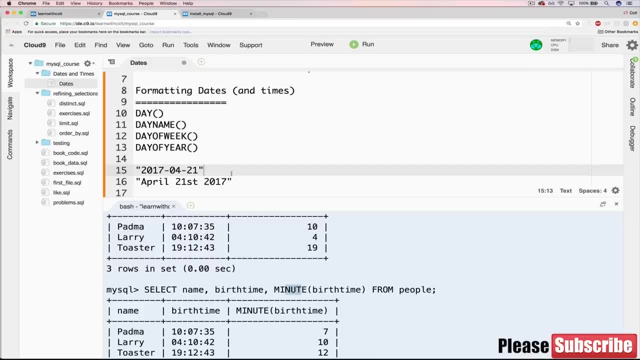 Well, we could use what we've already seen and do a giant concat. I won't make you do this entire thing, but basically we could extract the month, we could extract the month name to get this and then concatenate that with a space. 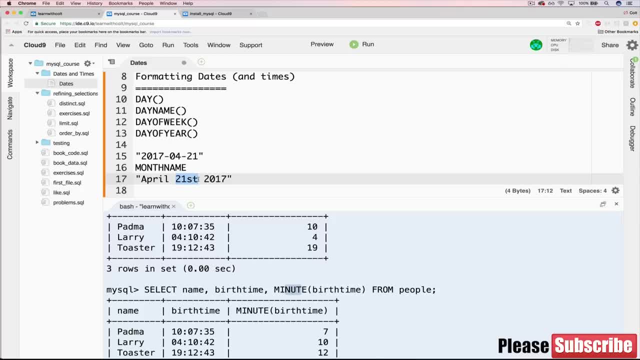 And then this part's a little trickier. right, We need to. it's going to be a pain. honestly, You would have to have some logic. that I haven't shown you how to do yet, because you don't always add st after a number. 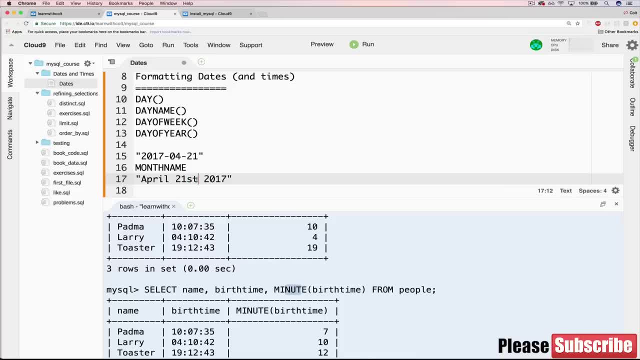 What if it's a 23rd? So that's a little bit more complicated, so let's reduce it to this. So for that we would want to get the day right, And then we want the year, So you could do a giant concat. 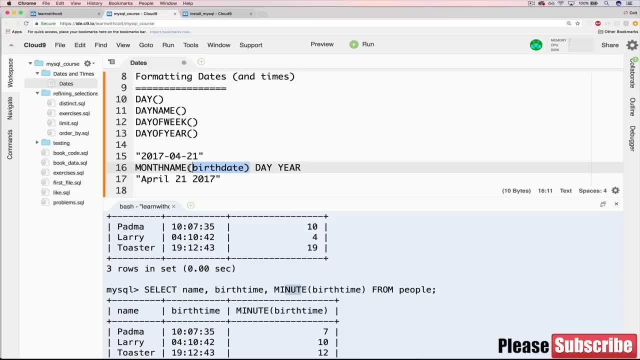 basically we would take all of these for birth date. This is going to get messy and the point is that there's a better way. But imagine you were doing this. So we have a concat month name of the birth date, comma with a space. 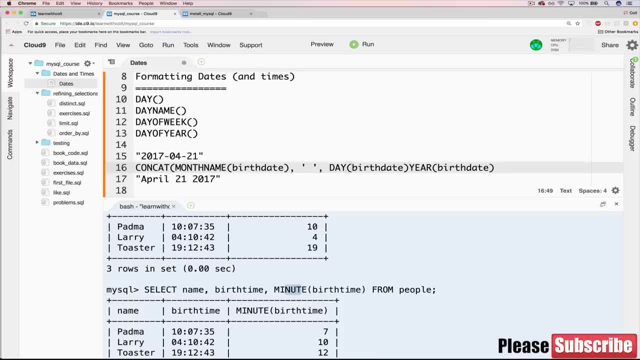 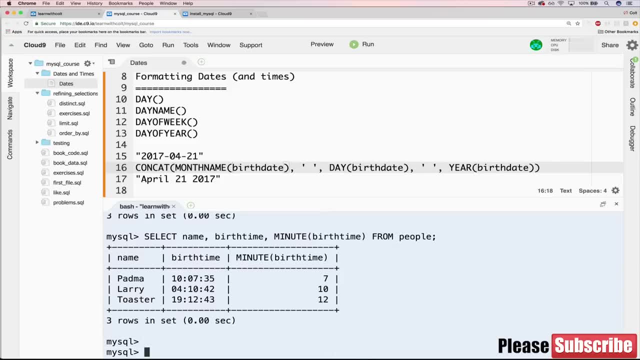 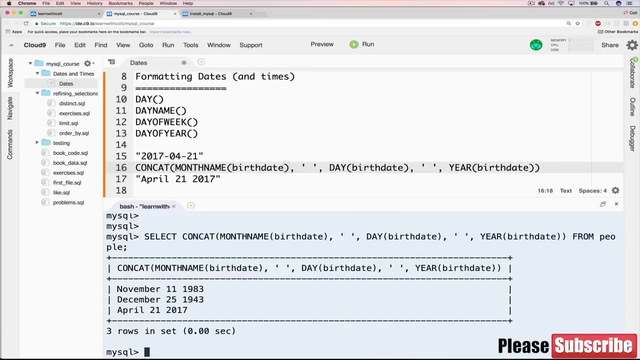 comma: the day of the birth date. comma. another space comma: the year of the birth date. It's a bit of a mess, But let's see if it does work. So we'll just select that from people. There we go. 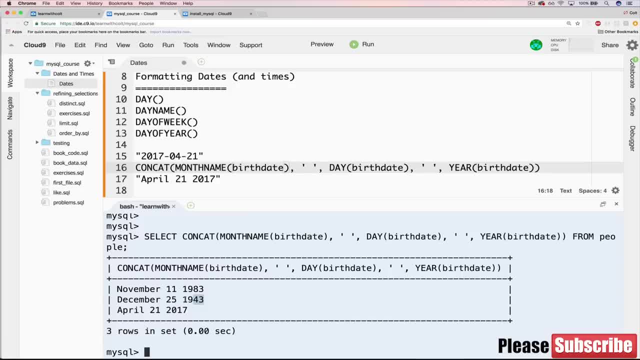 November 11, 1983, December 25, 1943, or 25, 1943, April 21, 2017.. So it does work, but this is not a great way of formatting dates and, in fact, 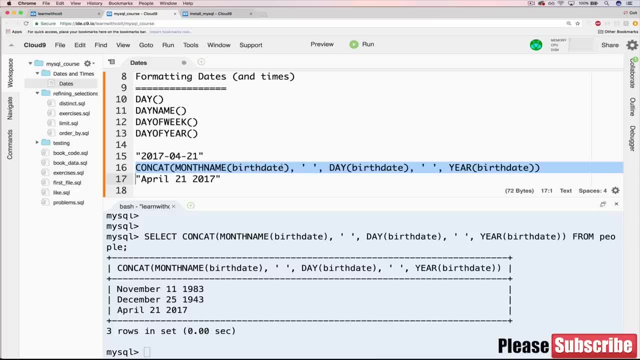 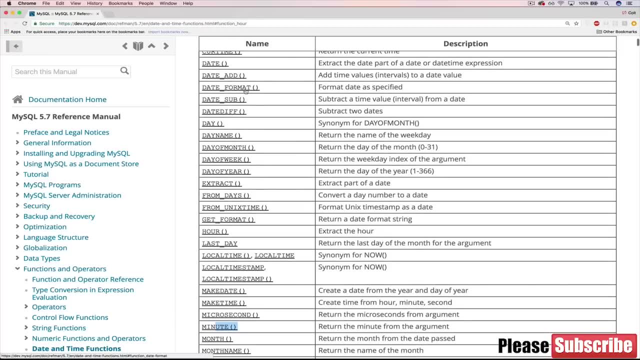 there's a better way, which you probably gathered because of the way that I set this up. There's an entirely separate method or function, excuse me, that we can use, which is called date format. So date format is really, really useful in my opinion. 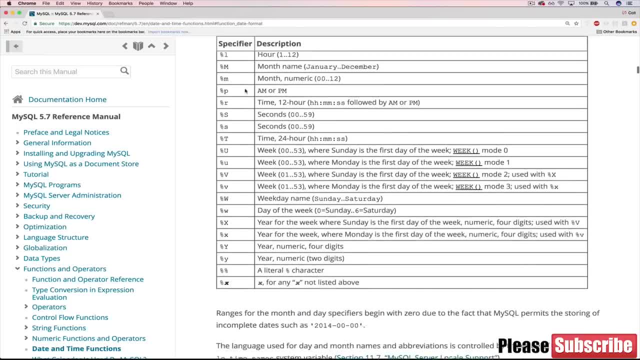 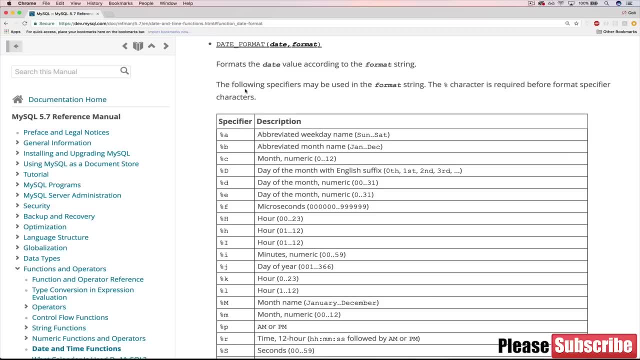 I use it all the time. What it does? it looks a little intimidating looking at the documentation, but what it does is it allows us to format things nicely and powerfully. We have a lot of different things that we can do, So these are called specifiers over here. 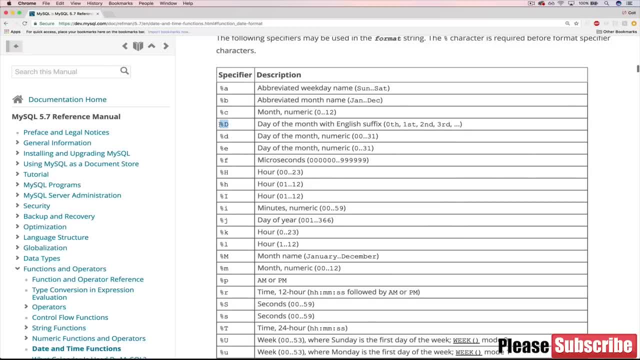 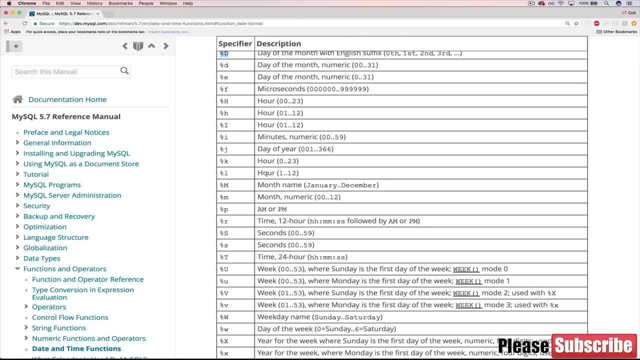 There's a table of them and they're basically little symbols, little shortcuts that allow us to specify what we want from that date. So let's say we're working with a date time and if I want to get the month name, I use percent sign capital, M. 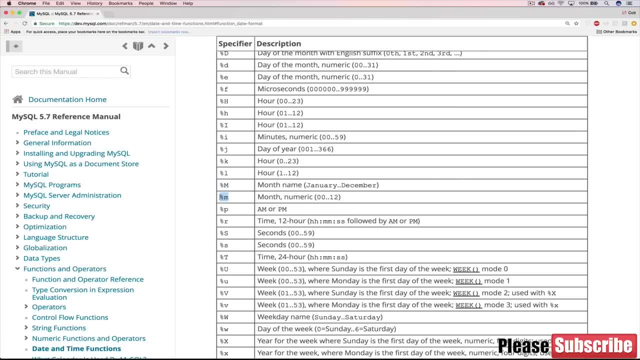 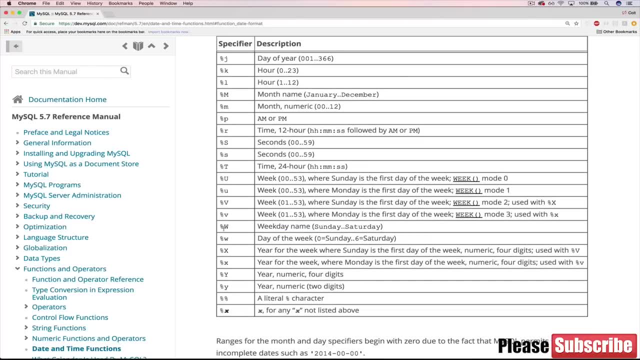 And if I want the month number, then I use percent sign lowercase m. If I wanted to get the day of the week as the weekday name, I use percent uppercase W. If I want the day of the week as a number, I use percent lowercase w. 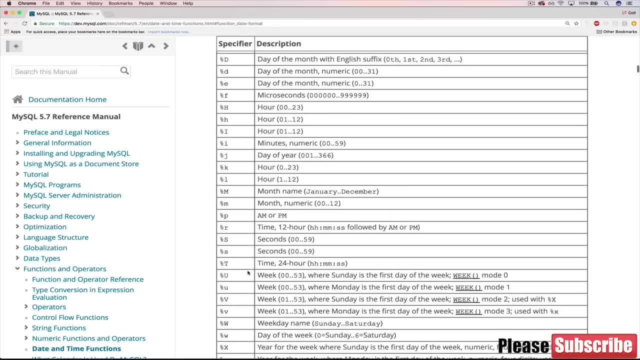 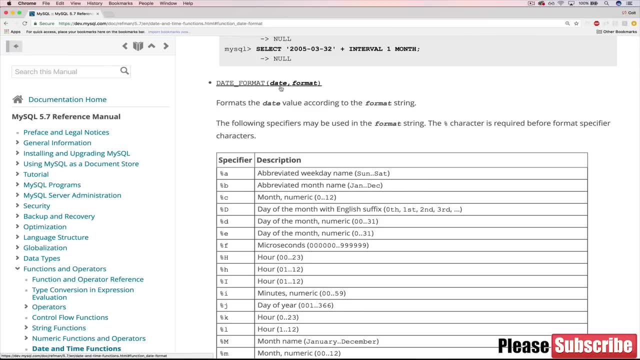 and so on. So what we do is combine them together in a string And when you pass it into date format, it will take a date and then the string of how you want to format it, and it will spit out a nice answer for you. 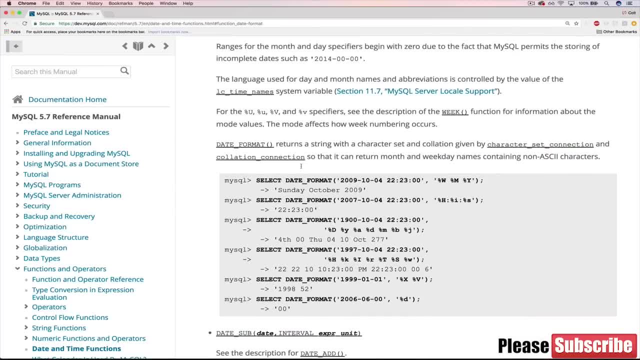 So here's an example. Excuse my fridge there, or my ice maker, I guess being noisy. So we've got date format of this date time here. It works on date times and just plain dates, So here's a date time though. 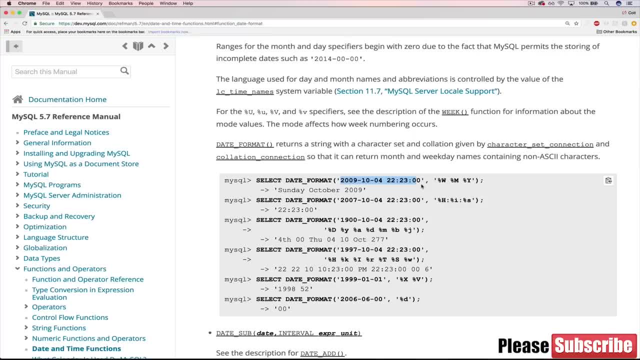 My fridge making so much noise. Okay, I think it's done. So we have this date time and we're formatting it with this, which looks a little bit like gibberish, But we have percent, uppercase W, which gives us the day of the week as the word. 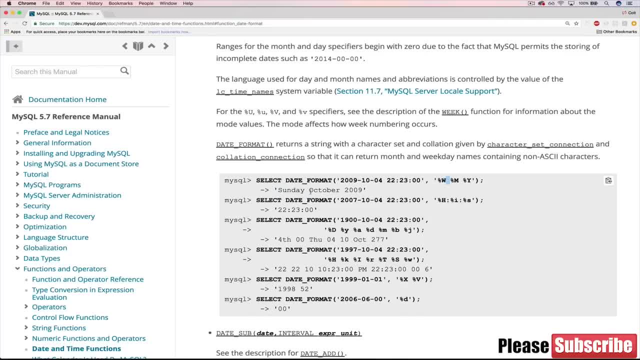 the name of the day of the week and then a space which gives us that space. Then we have percent uppercase M, which is the name of the month. So we have October and then another space and then we have percent Y. 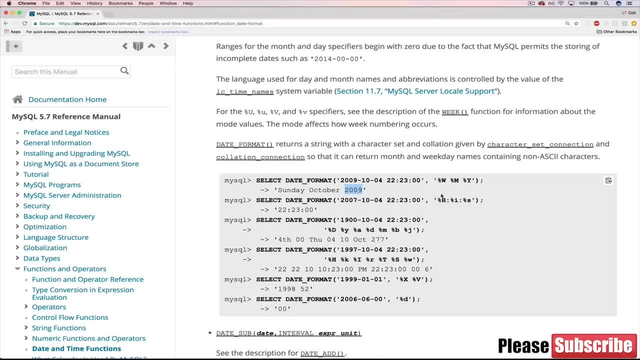 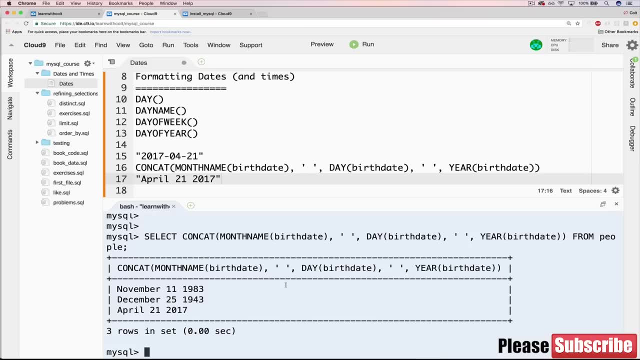 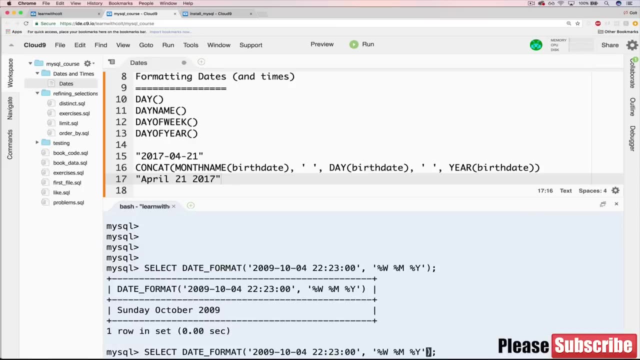 which gives us the year So really useful and versatile. I'm just going to just copy this one over, just run it so that you can see what happens. If I hit enter, we get Sunday October 2009.. But we're free to play. 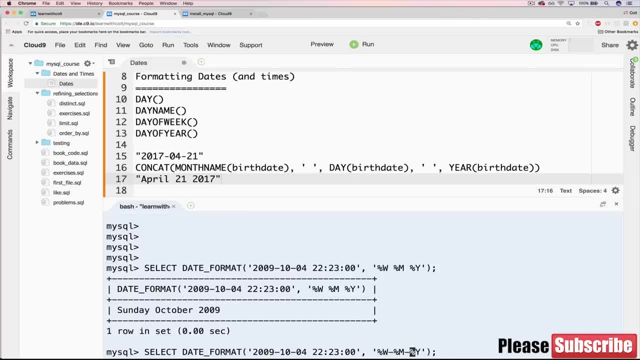 We can put whatever we want in here, So we can do dashes- not that it really makes sense. but if we put dashes there, it still puts the important information here that we specified, but now they're separated by dashes, So it gives us some freedom. 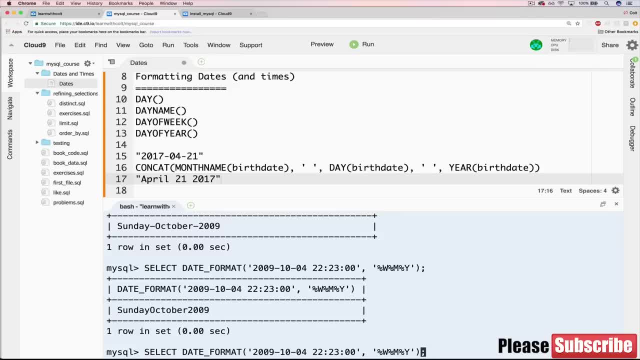 We can group them together like that, if we wanted to put commas, or we could put an entire word before or after, We can do whatever we want. So this is really really useful If we go back and select. let's work with date time. 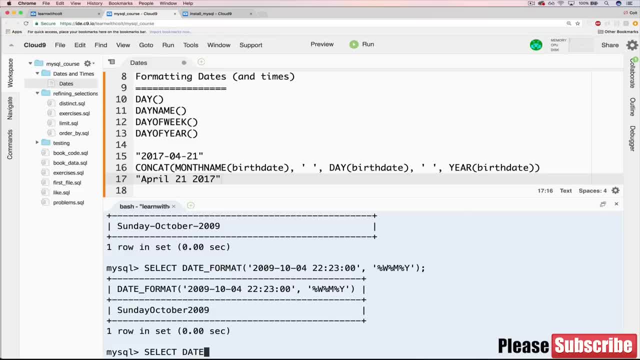 So we'll do select date format and then we're working with birth DT And then some string that we'll provide in just a second. We'll come back to that From people. We can start with something really simple like just getting 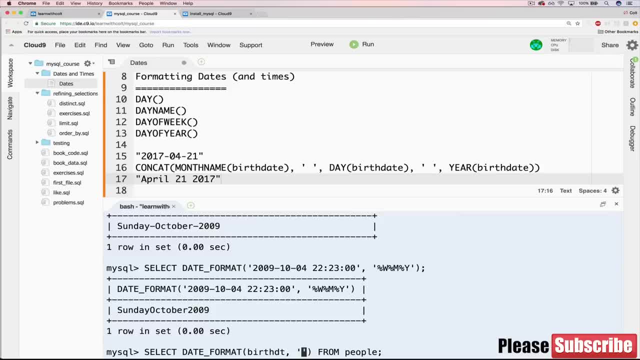 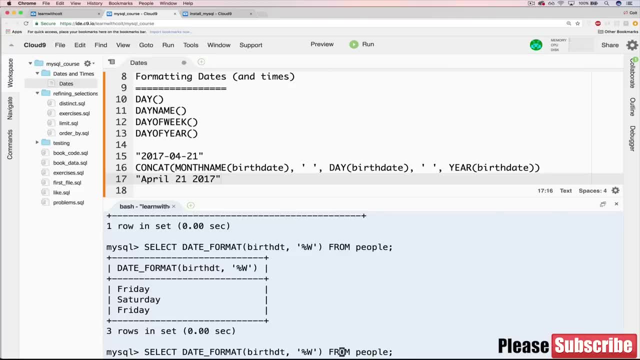 the day of the week as a yeah, day of the week first, as a word, So uppercase W. We could do something like was born on a Friday, Saturday, But, as you saw, there are a bunch of other things that we can do here. 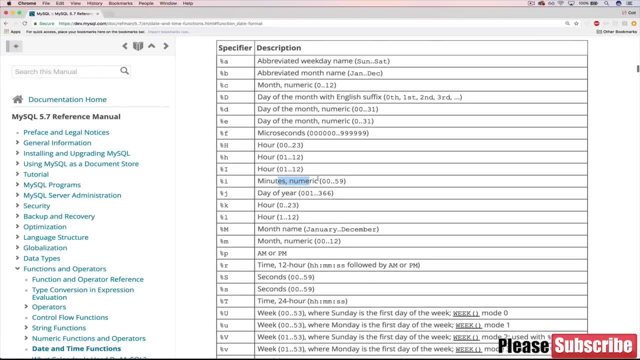 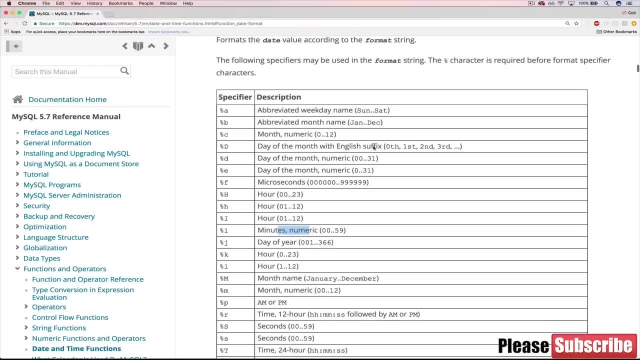 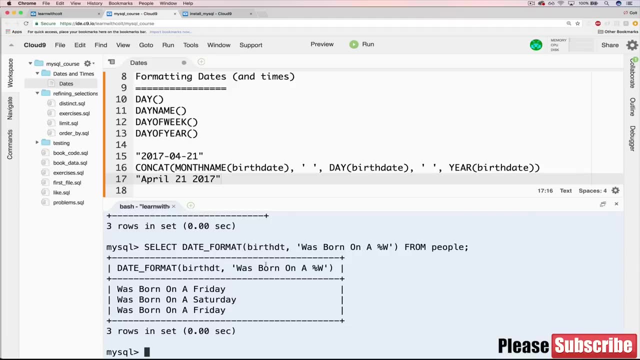 You know, we can work with hours and minutes, We can work with seconds, Month names, Tons and tons of things. It's really versatile and very useful And typically the things that I end up doing with it are just formatting dates so that they look like. 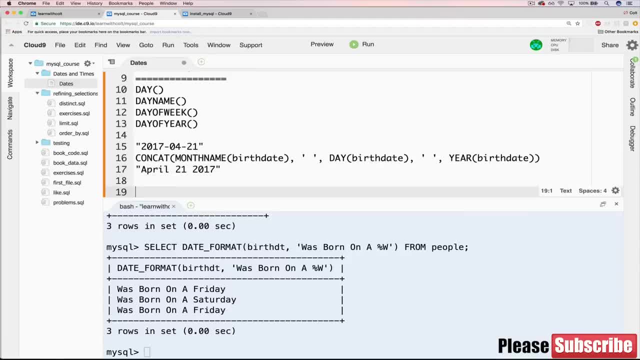 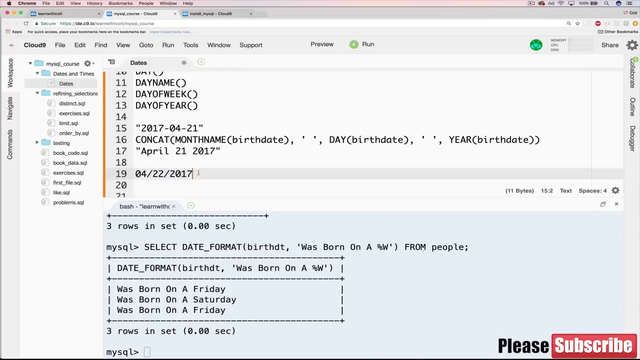 you know, at least in the US, where we put the month first, followed by the day, followed by the year, So that's pretty simple to do. Think about how you would do it, though. if you want to give it a shot, How do we take this and change it into that? 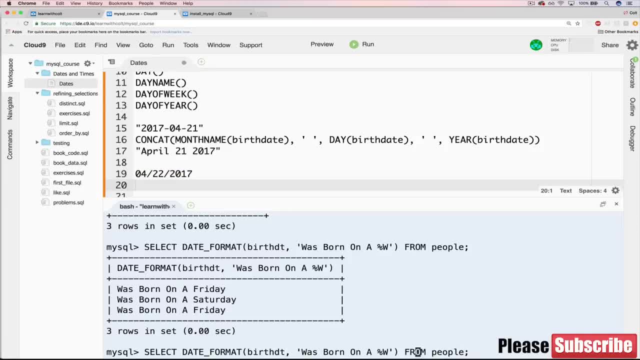 So we can do that now. All that we want is the month number, right? So that's percent m, I believe, Followed by a slash, And then the day, percent d, Followed by the year, which is percent y. 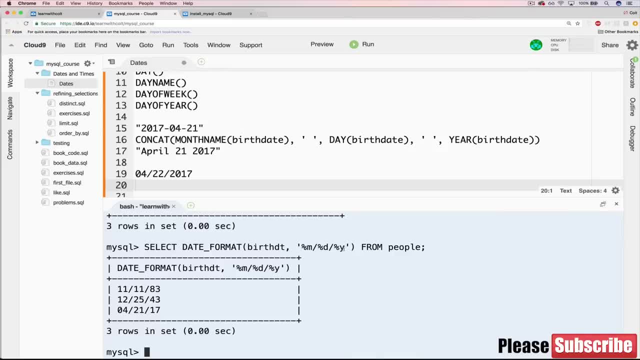 Let's see if that works Almost. If you notice, I use lowercase y and that gives us the two, that's the abbreviated year, the last two digits of the year. So we want uppercase y, And I just happen to remember that. 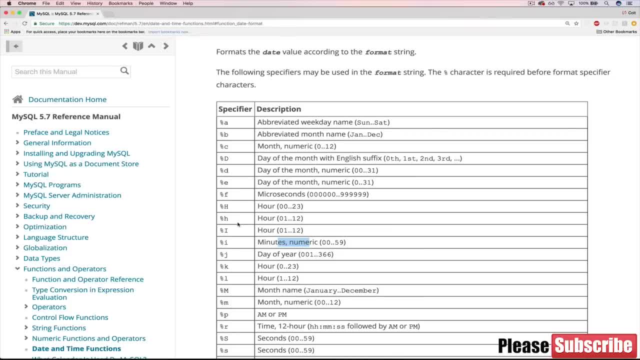 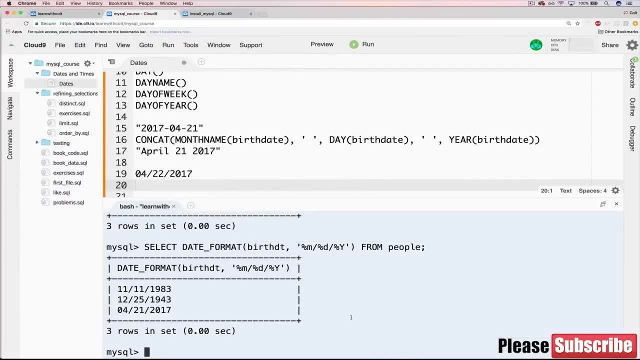 but if you couldn't remember how to do it, you can consult this And we'd find it. Where is that Year numeric? four digits versus two digits. So let's wrap all this up. We talked about a lot of different ways. 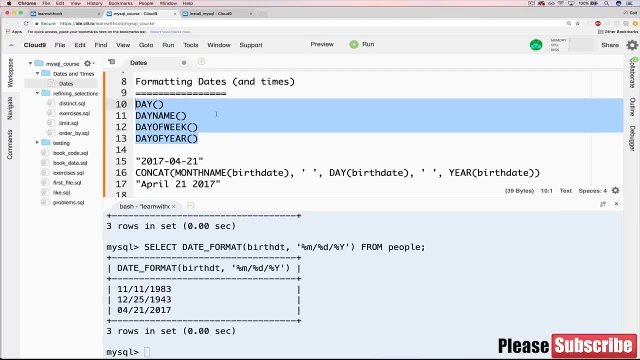 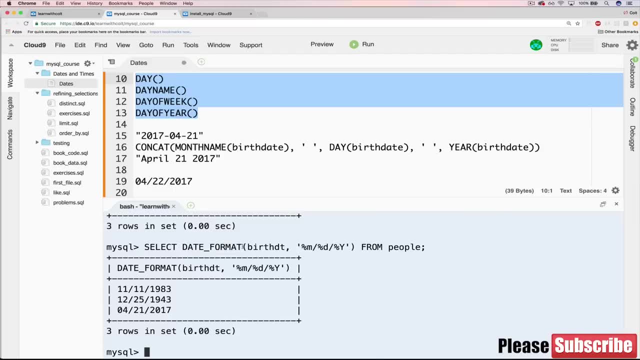 of formatting dates. I frankly don't use these that often, like I said, because you can do the same thing using date formats. I should mention there's also a time format. It works exactly the same way. You just pass in a different formatter here. 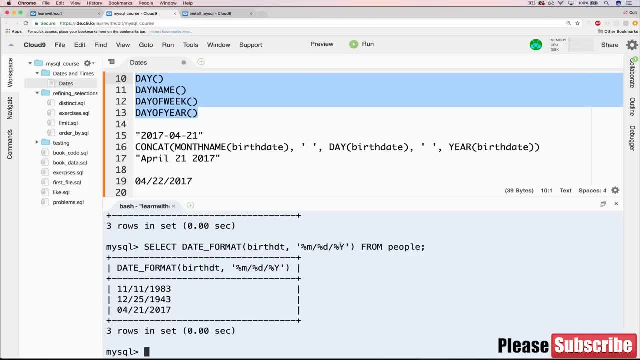 So you're not going to be able to get month, day and year from a time, but that you can get hours, minutes, seconds. But, like I said, I'm not working with times as often And if I am using a time component it's within a date time. 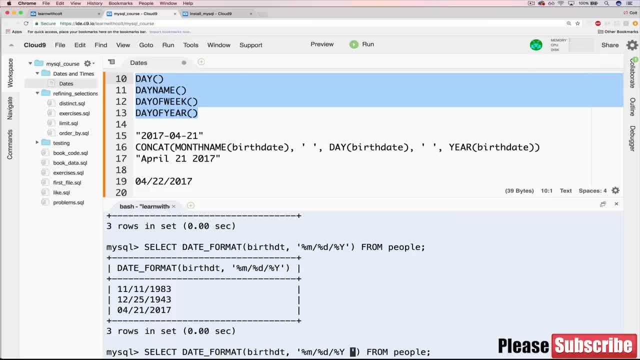 So I might do something like this At: and let's say, let's just do hour and minute And we'll put a colon there And there we go. So I'll do something like that, but I'm rarely working with just a time, but there is a. 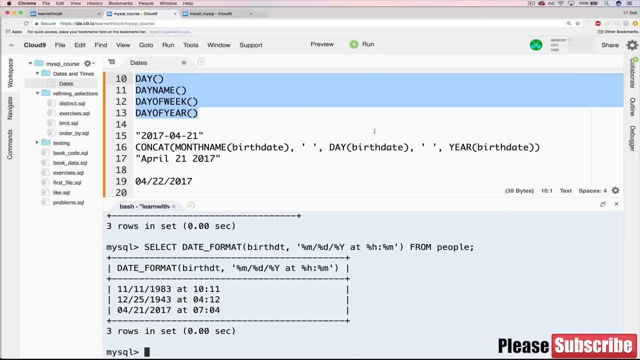 time format, if you do need to do that. Okay, so back to where I was wrapping up here. There are all these weird one-off functions. I don't use them, though, because you can just replicate it using date format, And it's much easier. 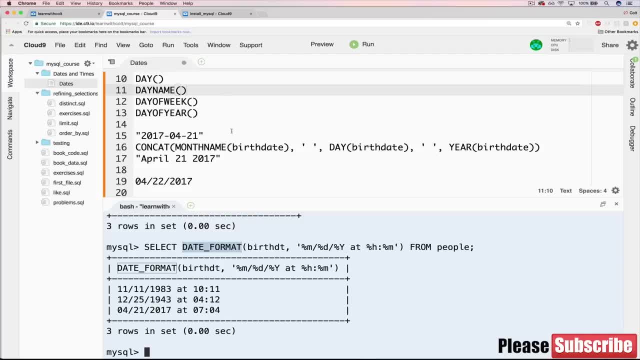 for me just to remember, one function- date format- rather than 15 separate functions. So that's the basics of formatting dates. Next up, we're going to talk a bit about doing math with dates. Alright, welcome back. So in this video, 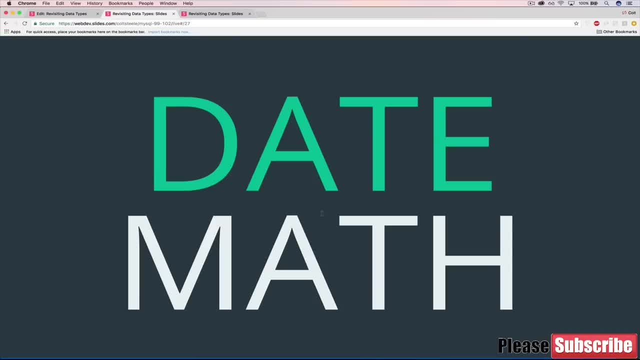 we're going to talk about date math. How do we add dates, subtract them, figure out how many days are between two dates, for example, Or how many minutes, Or take a current date and add, you know, 10 minutes into the future. 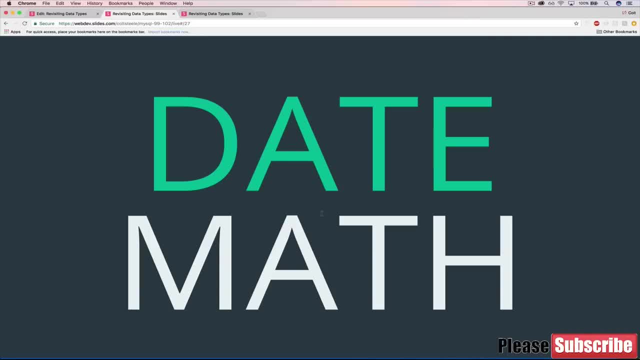 Or something like that. It's a pretty common thing to do, especially when you're dealing with comments or blog posts or some sort of information where it makes sense to display how long ago something was created On Facebook. I think I've been over this before, but Facebook. 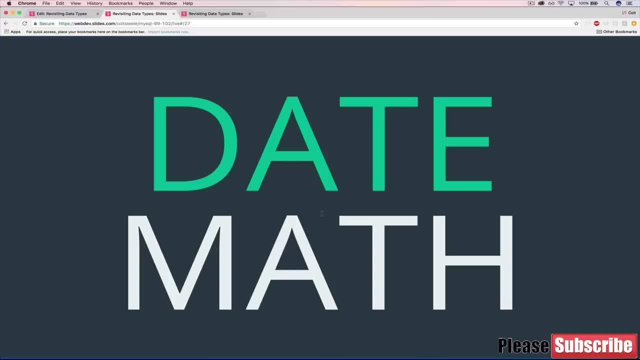 will tell you you commented on this 10 minutes ago. and then you come back the next day and it will say one day ago. And then a week later it will say a week ago, And then at some point it transitions over just to: 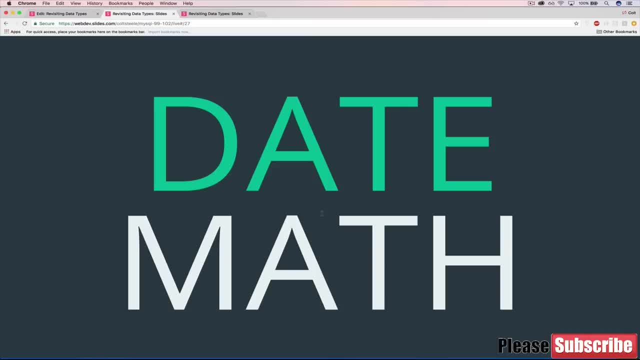 date. it will say December 5th or something. So you can accomplish that by using some of the tools I'm going to show you in this video. Now we're not going to spend a ton of time on date math, because it's not the most. 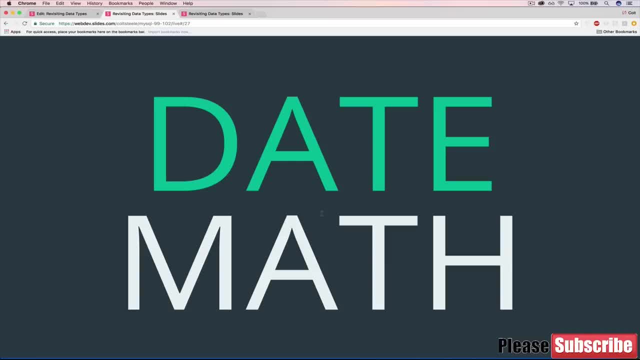 exciting thing Also. date math sort of sounds like you know, like at the end of a date, fighting for the check, figuring out who pays for what. Anyways, Yeah, it sounds like a bad band name or something. Date math though, in our case. 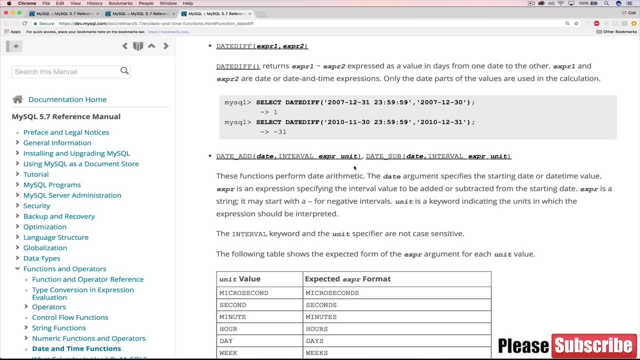 in our context, there's two main functions we're going to talk about, And the first one is pretty simple. It's called date diff, No underscore, It's just date diff. It stands for date difference And what it will do is it takes two dates. 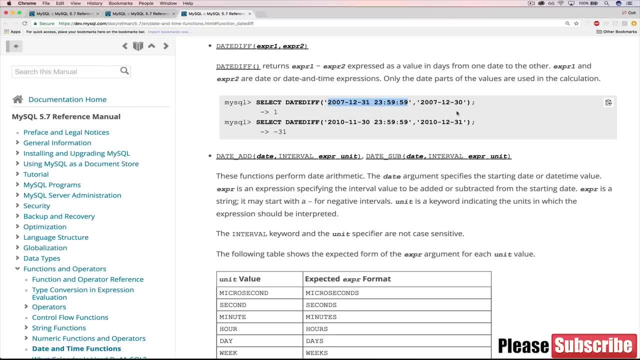 So here's an example One, a date time, Which I should highlight. pretty much everything in MySQL that has date in the name will also accept date time. So okay, here's a date, A date time, Excuse me. And then here's a date. 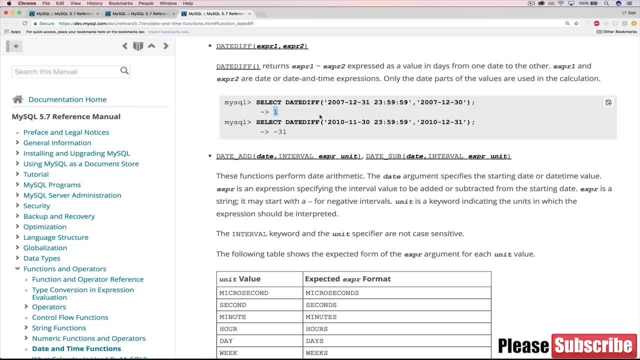 And when you subtract them, turns out they're one day apart. So this always tells you the number of days. So it's not going to give you minutes or seconds or months or something. It gives you days And then, if you wanted to, you could turn that into months or something. 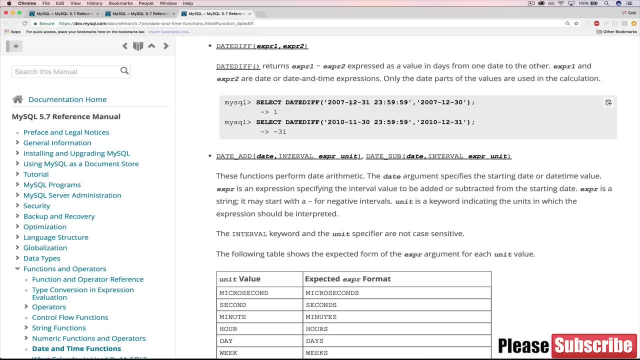 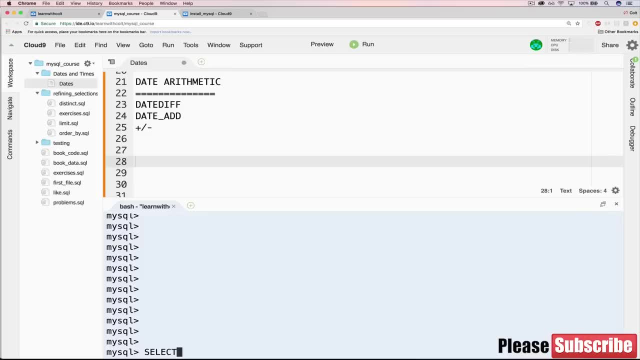 However, it's just. it's primary purpose is to give you the number of days, So let's try it. We could do something like this. Let's work with our star from people. Let's work with that And let's figure out. 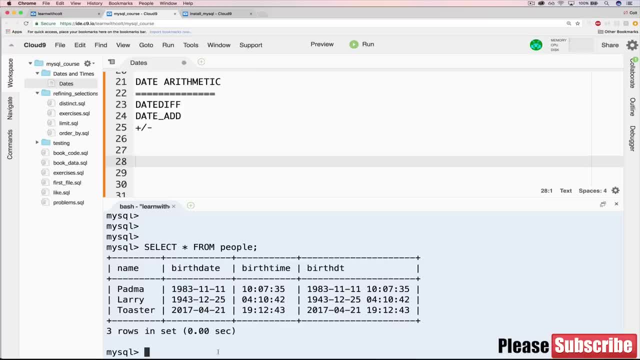 how many days ago each one of these, each person here, was born. So it would be something like select date diff And then we want to take now and subtract birth date. Hopefully that makes sense. We're taking now, We could. 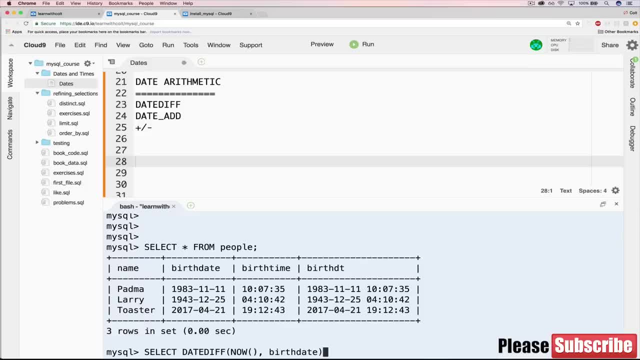 also do cur date. It wouldn't make a difference because we're not working with the time part, But I like now It's a short, easy to remember thing. So select date, diff now comma birth date. So that will take current date. 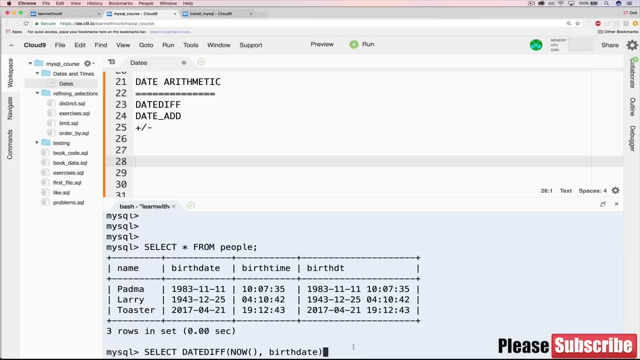 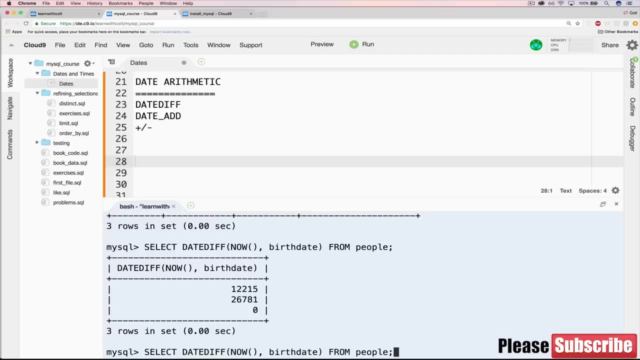 subtract birth date and find the number of days. Let's try it, Okay. So let's make this a little bit clearer. Let's do select date diff and we'll also display name and birth date. Here we go. So, Padma. 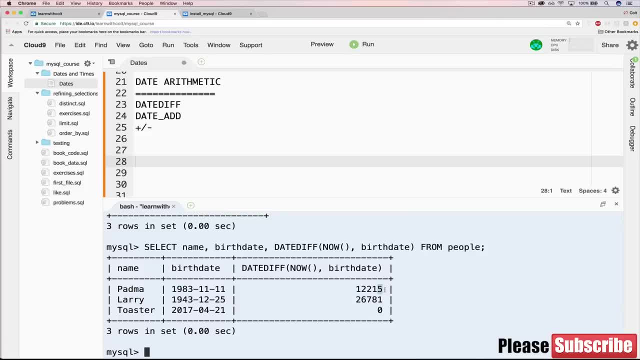 born in 1983, 12,215 days ago. Larry, born the longest ago, 1943, is 26,781 days old, And then Toaster, who was just born today, is 0 days old. Alright, So that's all there is. 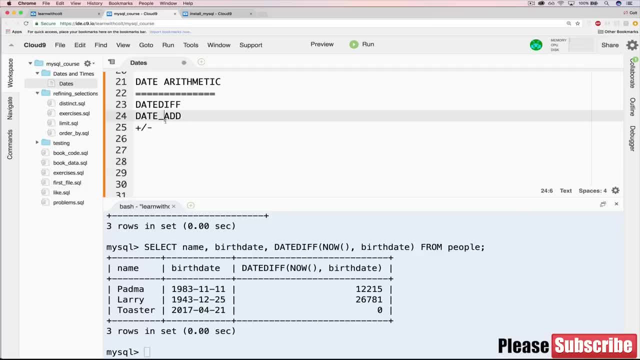 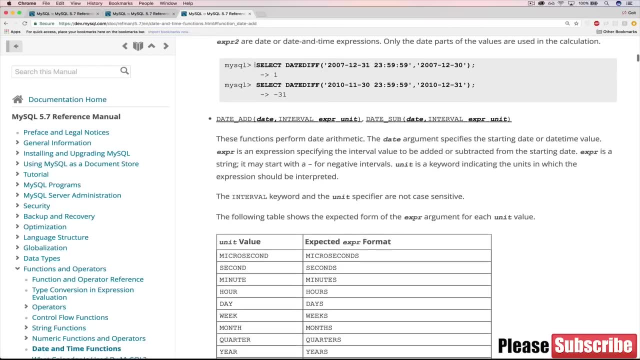 to date diff. The next thing we're going to take a look at is date add, And there's a little bit more to this to discuss there. If we just look through the docs, date add conveniently right below date diff, We get another table here. 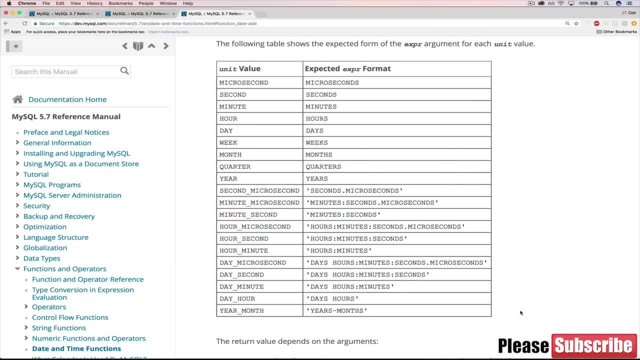 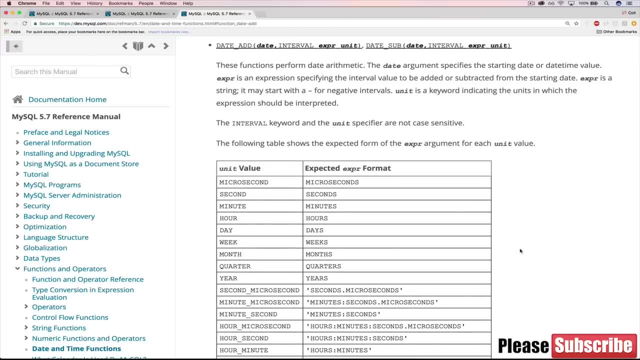 like we did when we had date format. There's a bit to discuss. So what this allows us to do, it is kind of the bread and butter for date arithmetic. So we specify a date, So date add. There's also. 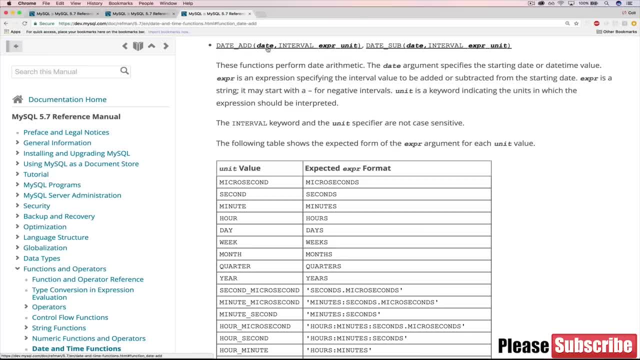 a date sub for subtract, but we're just going to work with date add for now. So we get a date or a date time and then a comma and then this sort of weird syntax that basically specifies what we want to add. Do we want to add 10 days? 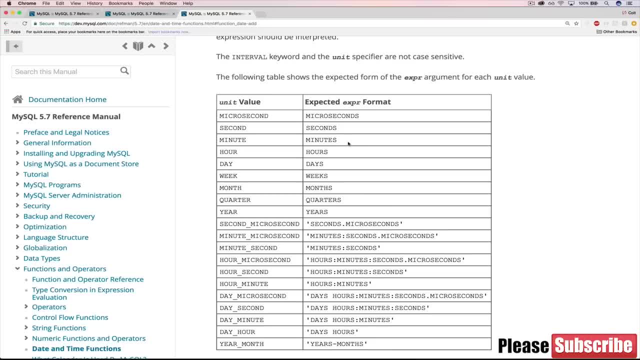 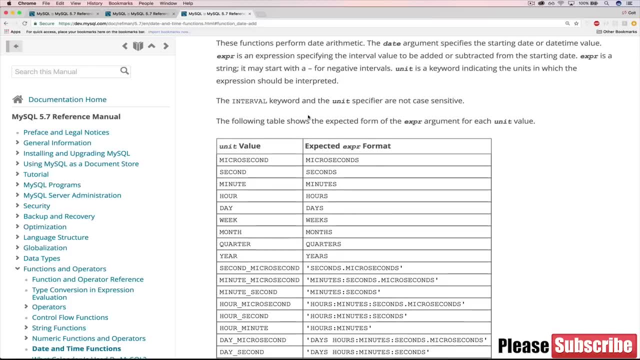 1 year, 4 quarters or 3 quarters? how about 18 months, 10 microseconds? whatever it is, the way that we specify it is using the interval keyword, And then we pair it with one of these units. 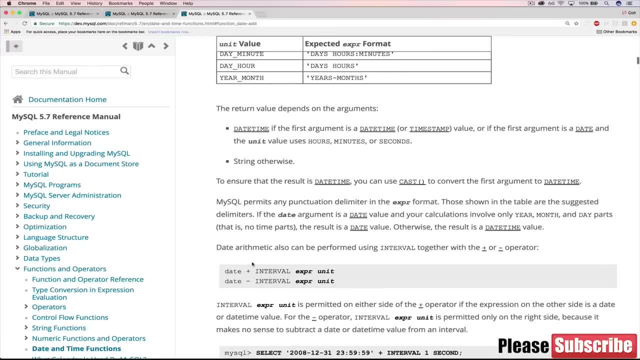 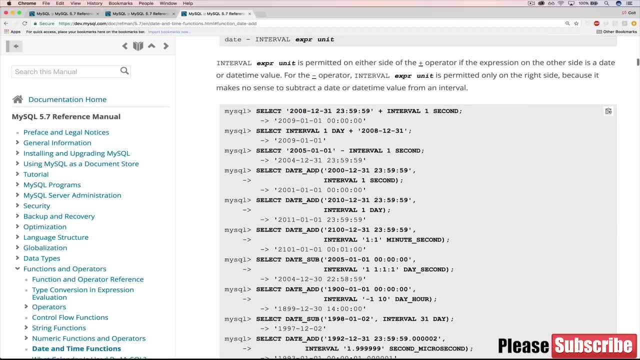 and then put it all together It looks something like this: So if we have this date time actually, let's take a look at this example here: Date add: here's a date time and if you want to add one second to it, 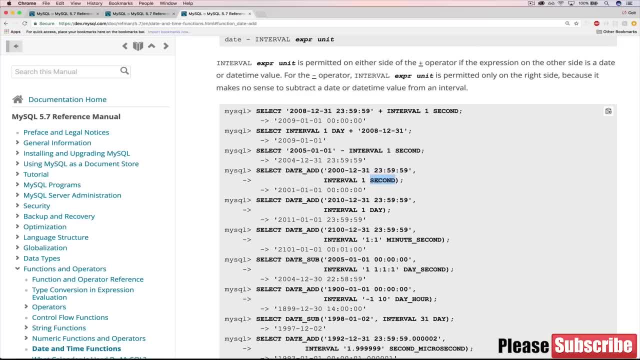 you just have to say interval and then second which is the unit, and then how many seconds. So it follows that format. Interval one day, And then it gets kind of weird when there's things like minute second. So this will do one minute. 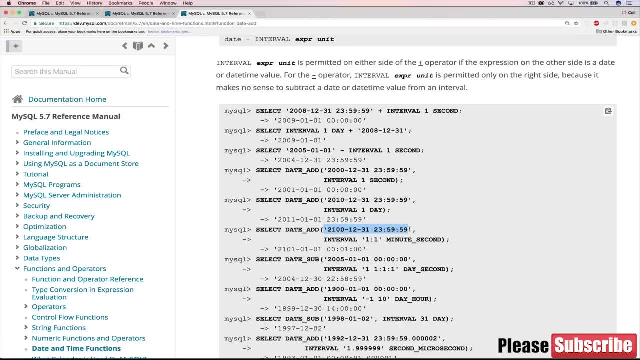 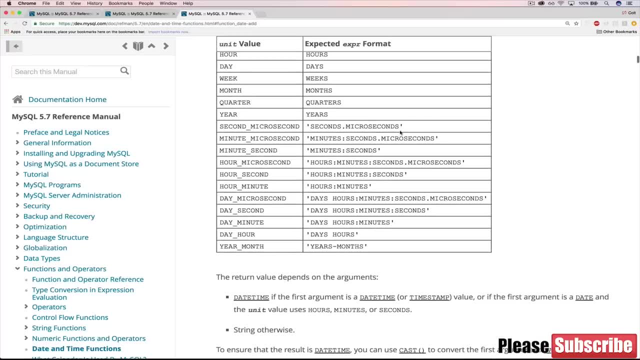 one second. add that to this date time. Pretty nuanced thing. I've never had to use these ever, But good to know that they exist. So let's give it a shot. Let's work with, let's do- why not? 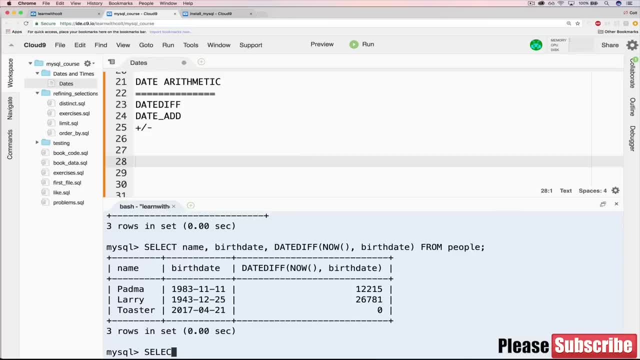 Let's do months, So we'll go here, we'll do a select and let's do date time this time. So select birth date time from people. just take a look at what we have. Alright, and now let's try. 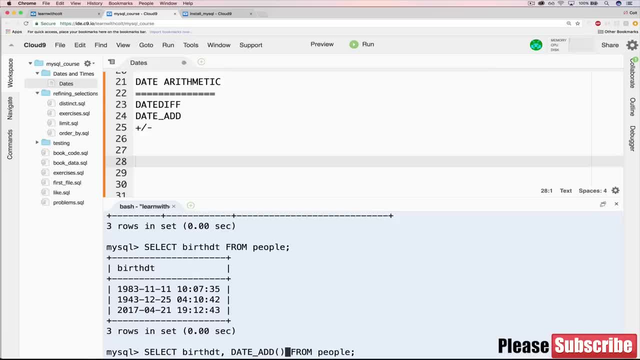 also doing a date- add birth date, time and we want to add one month. So we have to say interval one and if you can't remember you can go over here month. It's pretty straight forward, Okay. 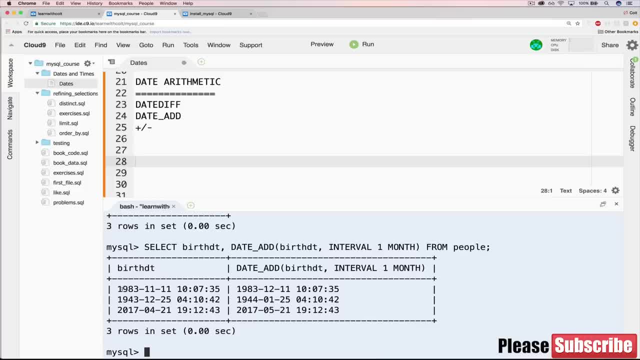 So, as you can see, here we go from 1983, 11, 11, to 1983, 12, 11.. Or here, 1943, 12, 25, here's a significant month. 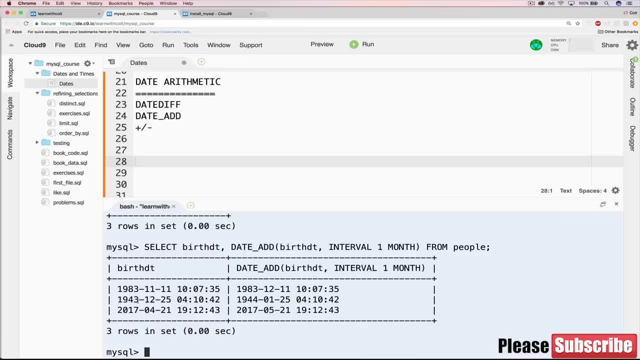 We went from Christmas of 43 to January 25, 44. So we can also change that over and do things like: rather than one month, what about 10 seconds? You'll just have to trust that that works. We can look at it. but. 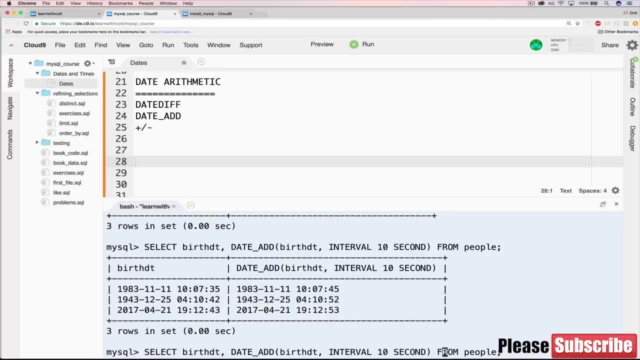 I won't spend time in this video doing that. We could also do things like 3 quarters And you might be wondering: okay, that's great. what if I wanted to do multiple things, Like I wanted to add one month and a year? 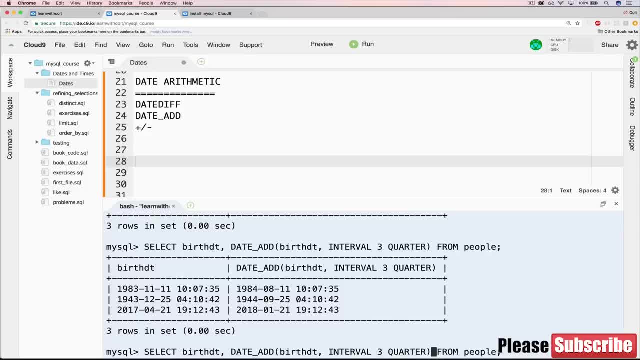 Or I wanted to add, I don't know- 10 years and 2 seconds. Well, the easiest way to do that is with two separate date adds. There's no, you can't just chain them together like this. You know 2 seconds. 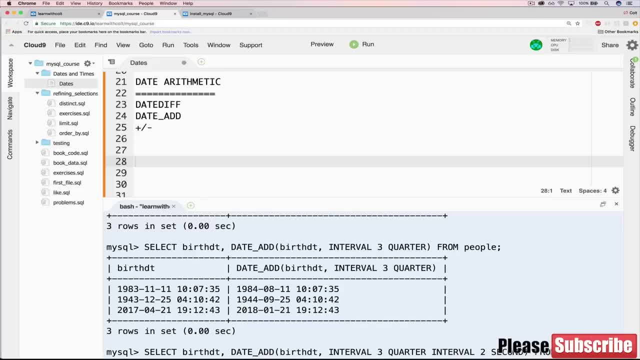 or something That doesn't work. However, there's a nice shortcut that I'll show you right now, Which brings us to our third way of doing date arithmetic, which is just with the plus and minus sign. So if we go back to the docs, 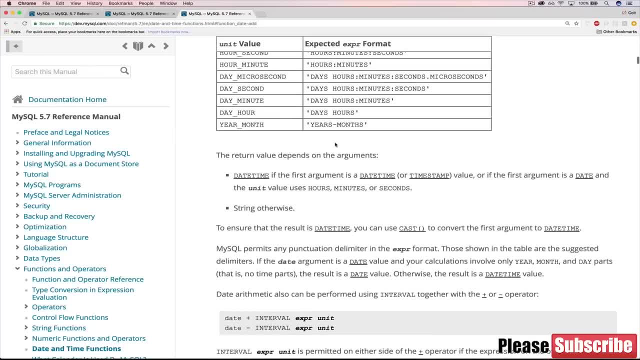 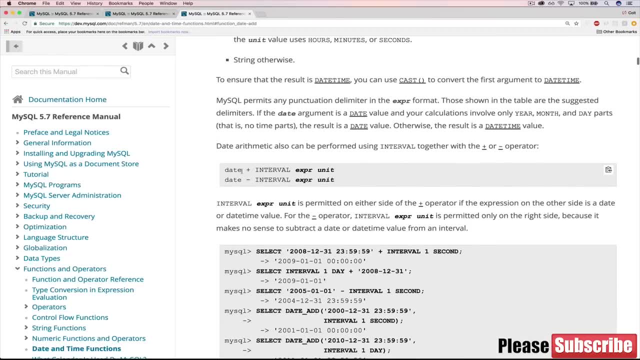 you can actually see that, rather than using date add or date sub- which I didn't go over, but it works the same way as date add, except it subtracts things- You can just use a date and then the plus sign and then the interval. 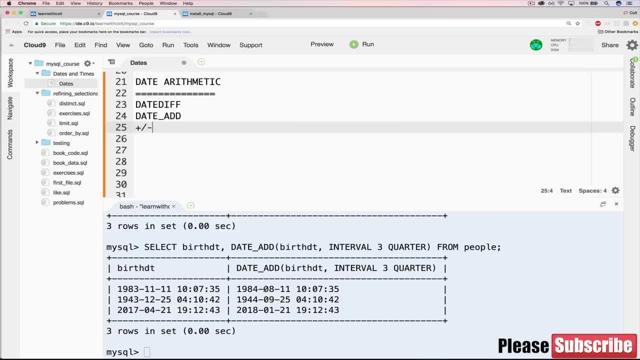 expression and a date and a minus sign, So we could rewrite what we did at as if I go back here, this one where we added 1 month, All I need to do if I get rid of the date add. 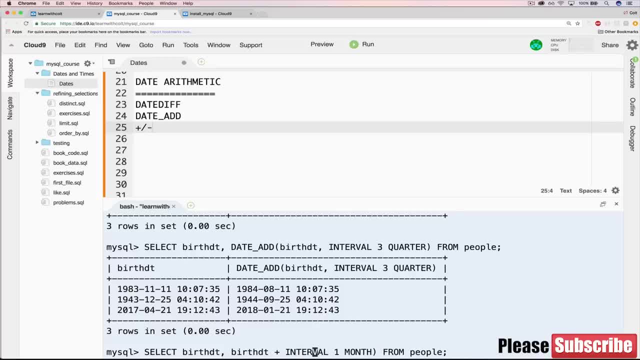 is just do birth date time plus sign interval 1 month. As you can see there it still works. Or I could do subtract 5 months And this takes us back 5 months, 5 months and 5 months. 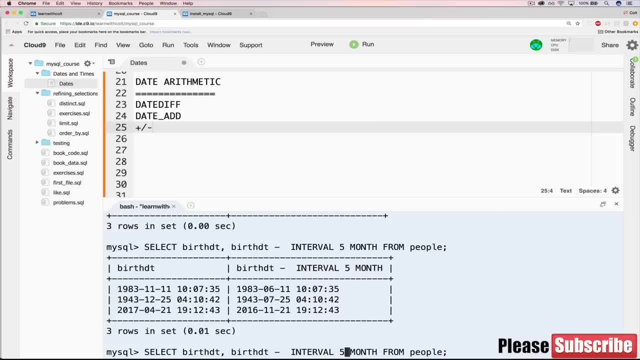 Alright, So the only other thing that will show is that you can chain them together this way, So that you could do something like take a date time and add interval 15, month plus interval 10, let's do hours. So, and if you take a look, 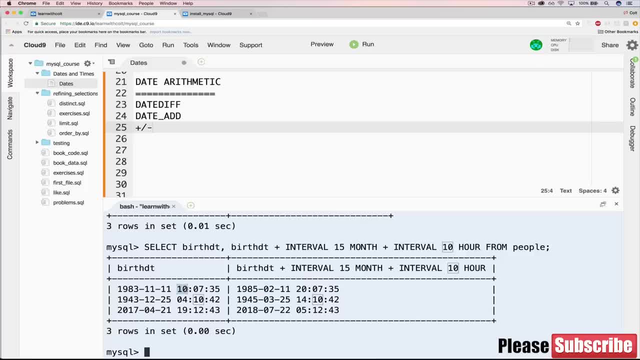 we're not only adding 15 months, but if you look at the time portion, we went from 10 to 20, 4 to 14,, 19 to 5.. So we're adding 10 hours successfully, So. 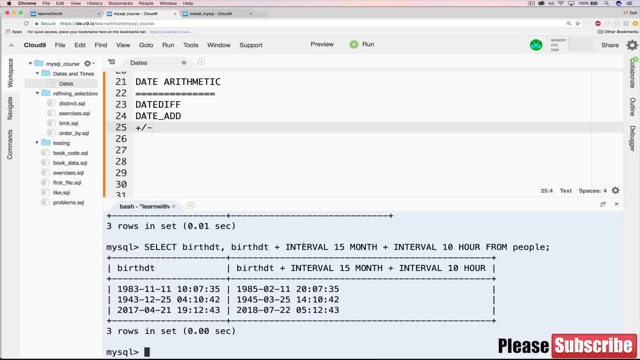 this is the. this is my preferred way for doing date math. I will say, though, it's not that often that you're doing things like adding 15 months or adding 10 hours. Often, more often than not, I'm actually using date. 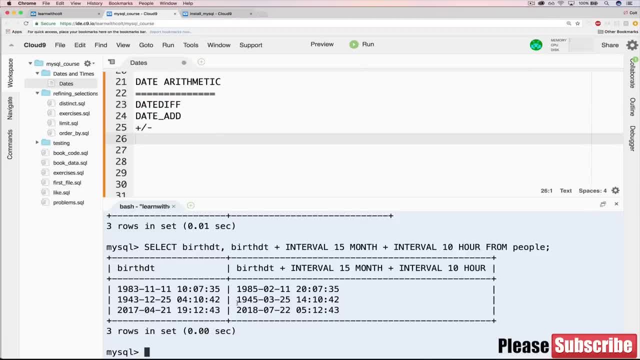 diff and finding how long ago things were relative to now, relative to current time. Okay, so that's pretty much it for date math at this point. The last thing that we're going to talk about in the next video is how we set up timestamps. 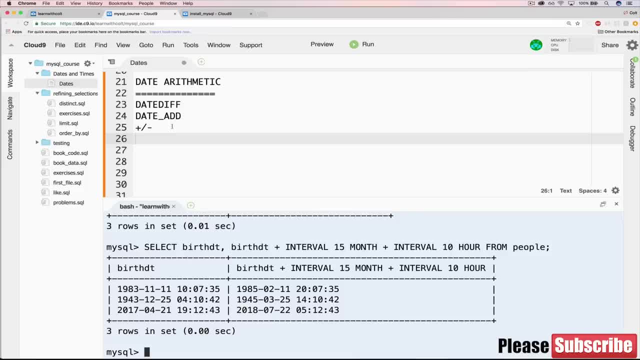 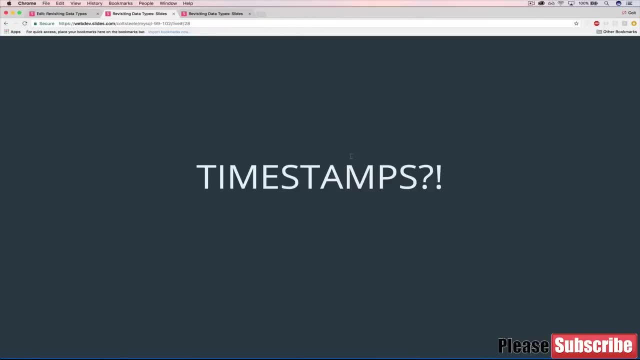 So a new topic: how do we automatically store, when a row is updated, what time it was updated at? So we'll see that in just a sec. Alright, so this is the last bit of new content around dates and date times and times. 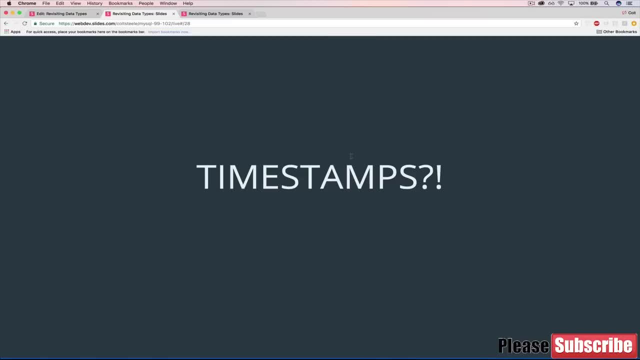 I admit that this section is a bit of a doozy or a pain. I don't know, Maybe not the most exciting thing. With that said, this is a really important topic that we're going to discuss here, And it's something that you'll be. 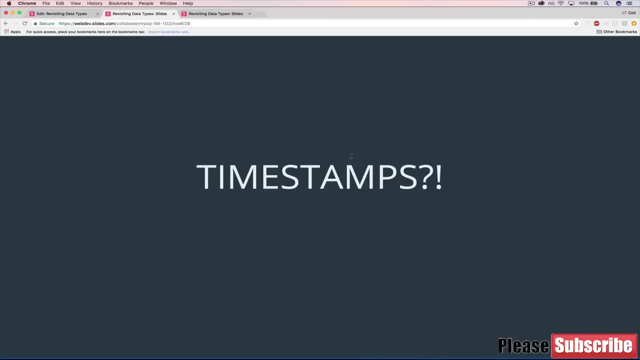 doing all the time, or probably will be doing all the time- I do it all the time- Which is adding in timestamps to our tables. So when we say timestamps, there's two things to unpack. One is that that's a generic term, that just 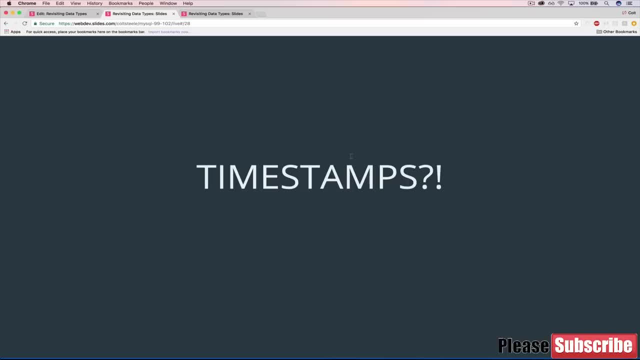 refers to storing information, metadata about when something is created or updated at It's sort of a standardized name across programming languages or across just in programming in general and app development Timestamps. refer to basically saving information about when you create a post or when you insert something into. 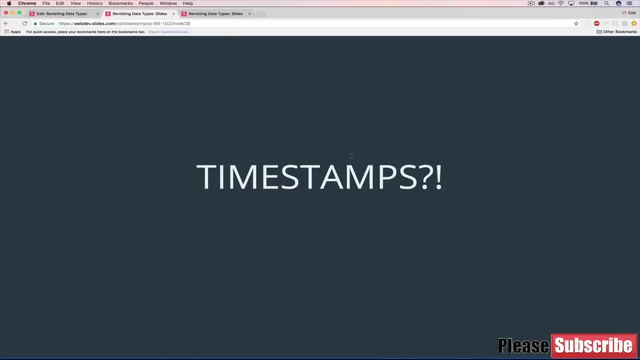 a table. However, in MySQL, timestamp is also a data type. So yes, I know it's the last video in this section, but I'm actually going to show you another data type, So hang in there. Fortunately, this. 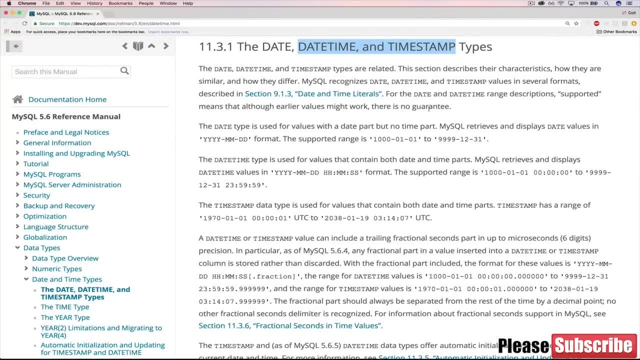 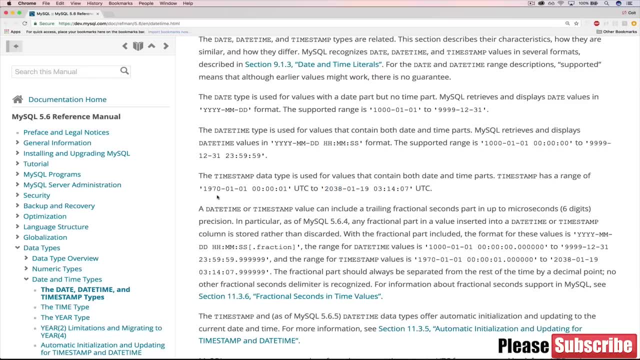 data type is really simple and there's only one case that I recommend that you ever use it. Okay, so there's a page called the date, datetime and timestamp types. We're going to ignore date. we've already talked about that. Let's compare. 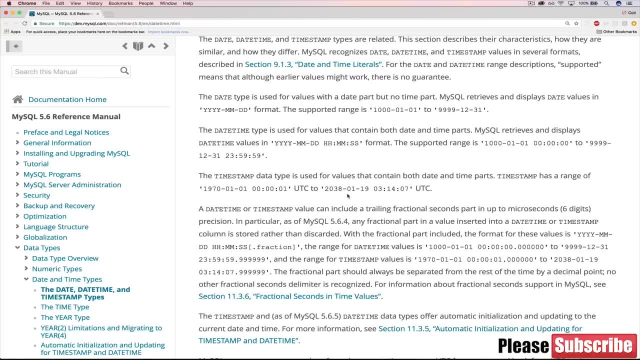 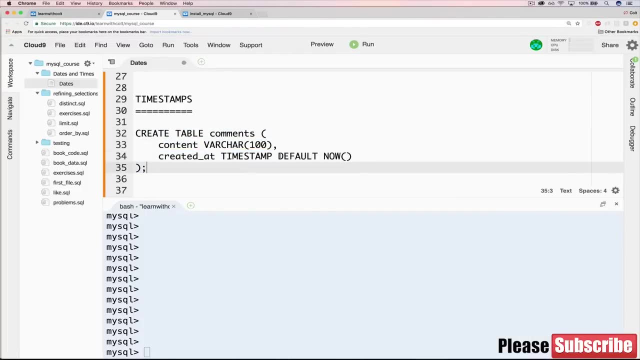 datetime and timestamp. They both do the same thing: They store date and time information, But there's two differences If we read the description. datetime is used for values that contain both date and time parts. Yes, we know that. The timestamp 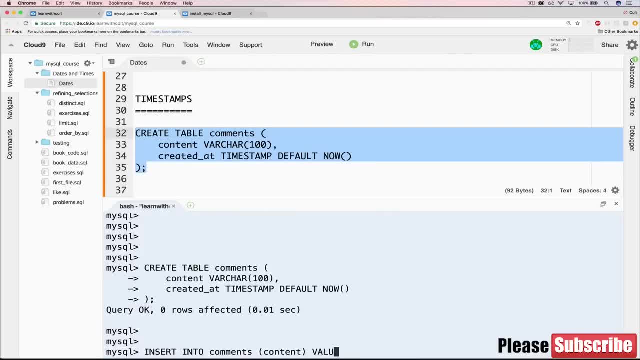 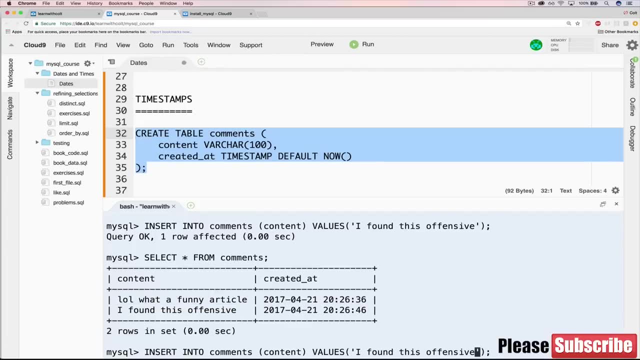 is used for values that contain both date and time parts as well, So they're identical in that sense, But the main difference comes down to the range of times and dates they support. So if we look at datetime, it goes back to year 1000. 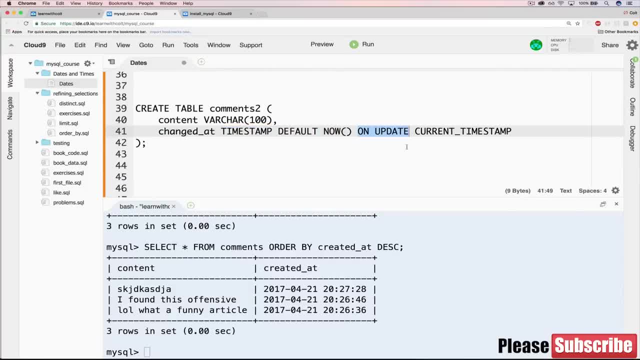 and all the way up to year 9999.. Timestamp, on the other hand, only goes back to 1970 and up to 2038.. So that's really important to note If you are working with something where you're storing dates that may go back. 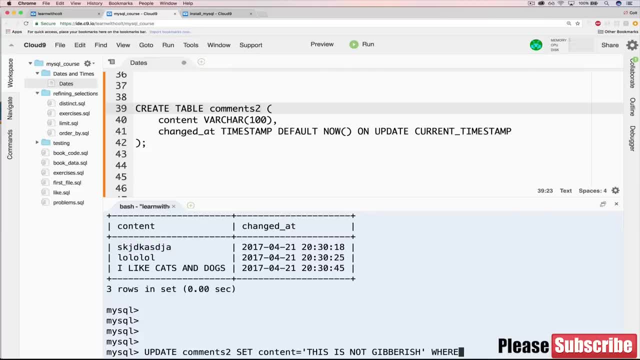 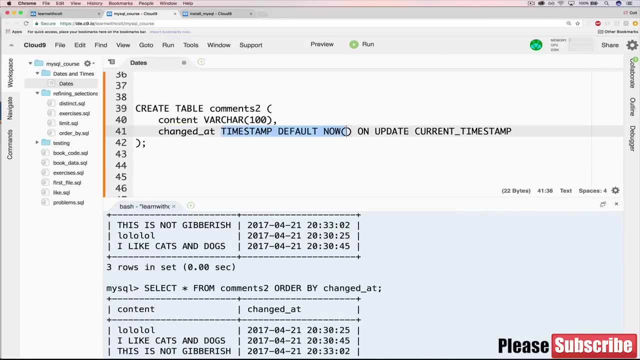 very far, like if I'm trying to think of a good example, but things before 1970. certainly you might have sites where you're storing a birth date and you might have users who are older than that and they're born in the 60s or the 50s. 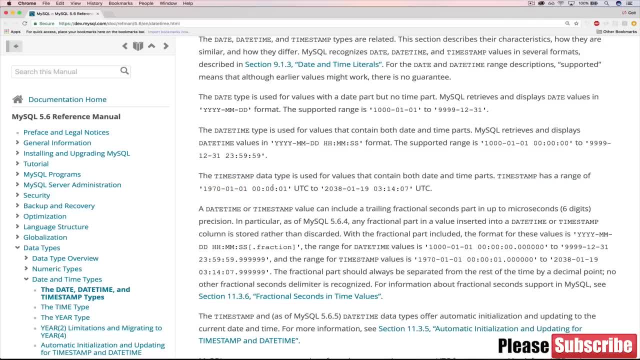 So timestamp would not work. Same thing going forward. If you're working with dates and datetimes where you need things to be further into the future- past 2038,, then you're not going to want to use timestamps as well. But for what we're talking? 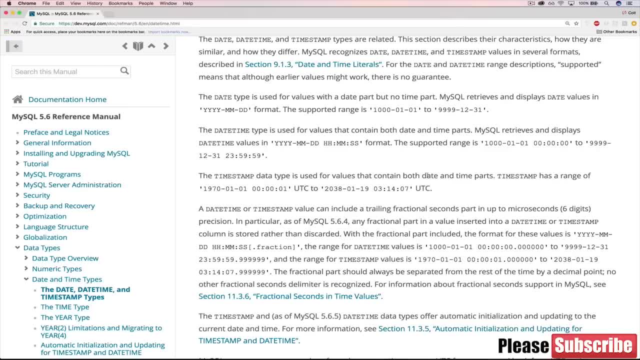 about just saving when something is created or when it's most recently updated. we don't need to worry about that being before 1970 or after 2038, because it's right now or when our app is up and running. now is relative. 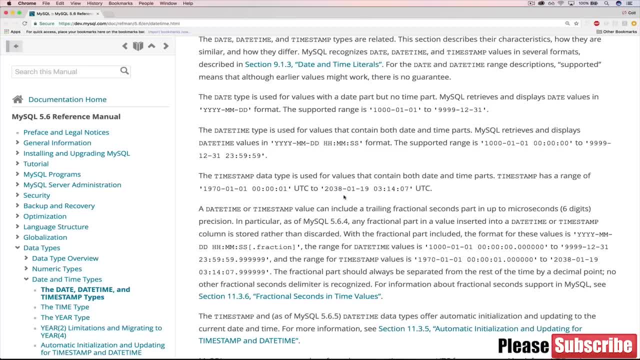 But basically it's not going to be past 2038.. And we're not changing those dates. All that we're going to do is store information. So timestamp is a good data type to use there. You might be wondering why use it in the first place. Why does it exist? 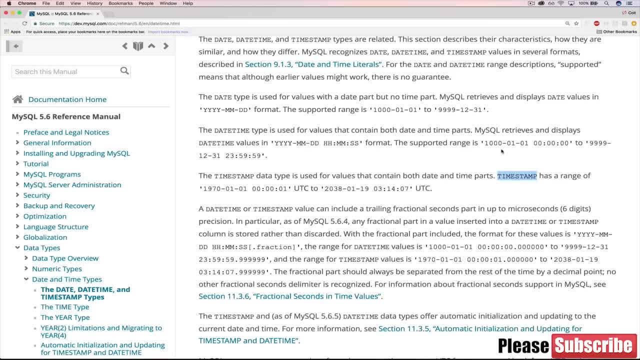 if there's already datetime. The answer, like so many things in MySQL, is that it just takes up less space. I believe it's 4 bytes compared to 8 for datetime, Or it might be it's double to use datetime compared to timestamp. 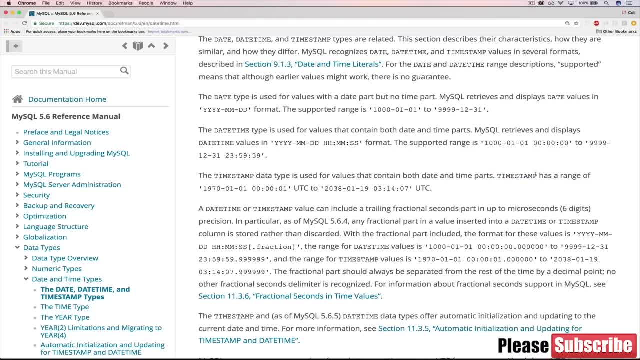 I believe it's 4 and 8.. So it's easier. and if you're doing something- every time you insert something into a row, you are updating something. That 4 versus 8 makes a difference if you're working with thousands and thousands. or millions of records. So now that we've got that out of the way, just to summarize, they store the same type of data. This one is smaller, Timestamps take up less space, but they have a more limited range. So use datetime for everything. 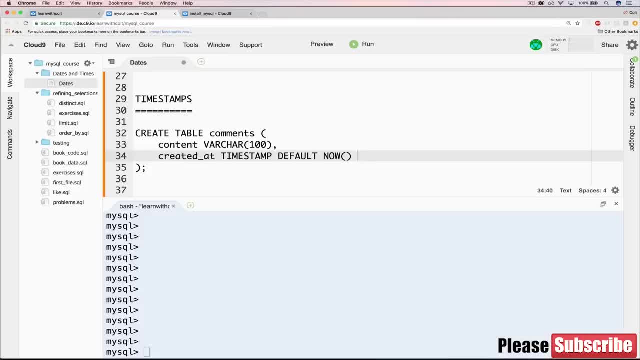 except for what I'm about to show you. Okay, so let's hop over to Cloud9.. Here we are, And I have a simple schema going to create a table called comments. Comments is very simple. It has two fields. The first, 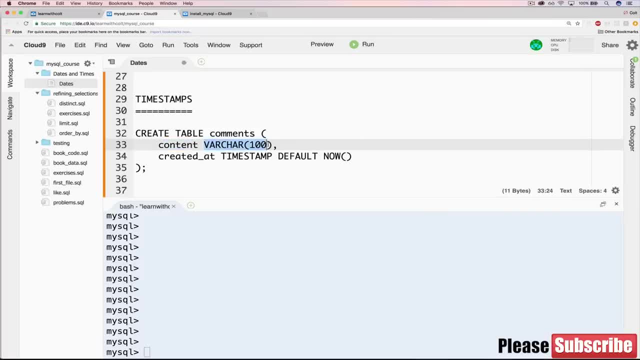 row is called, or the first field is called content, and it's just the content of the comment. You know things like great article, or I made a thousand dollars a week working from home. Learn how, Email me, Or whatever. 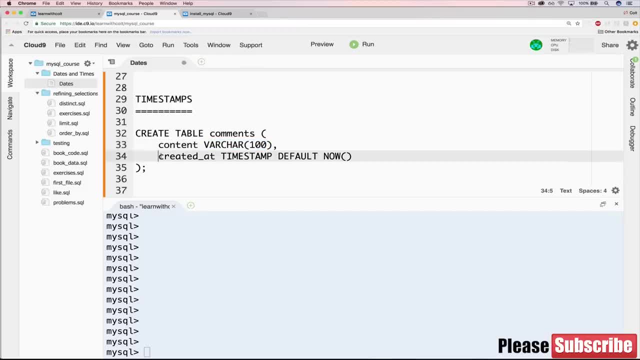 spam comment there is. And then this is the important part- What is it created at? Which is the timestamp? First thing to notice? It could be datetime. Just want to make that clear. You can do that, It will work, But we're using timestamp. 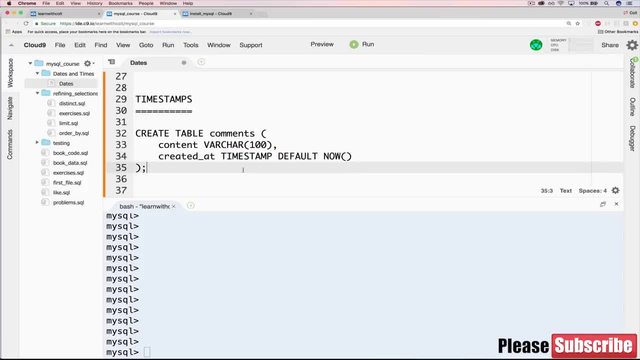 because this is basically what it's intended for And it takes up less space, So just setting it to timestamp on its own is not that useful. This is the key part: Setting the default value to be now, So whenever it's created. 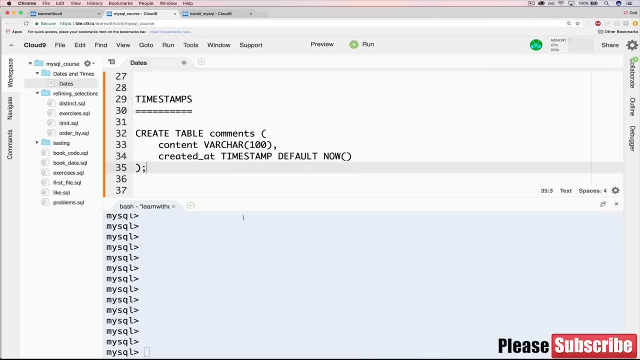 take that now, that current time, and put it in timestamp. So if we run this schema right now and we insert a few things, So let's do insert into comments. All we need to insert is content, And what we'll do is just: 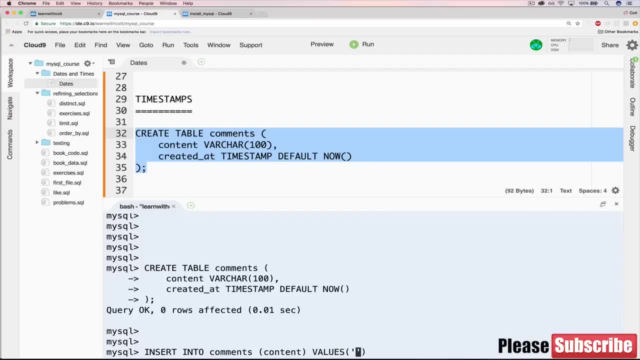 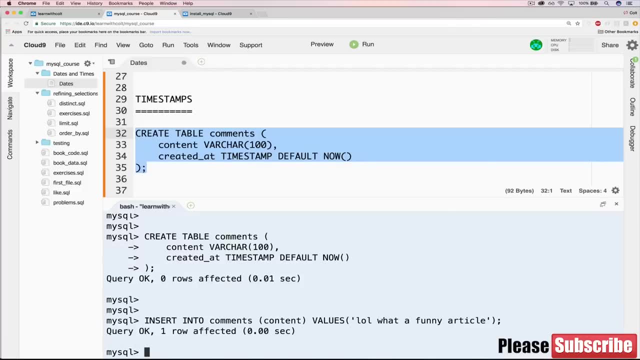 insert our first one. I'm going to do them separately so that they have different timestamps. So the first one will be: lol, what a funny article, Something silly like that. Then let's do another one Like um, I found 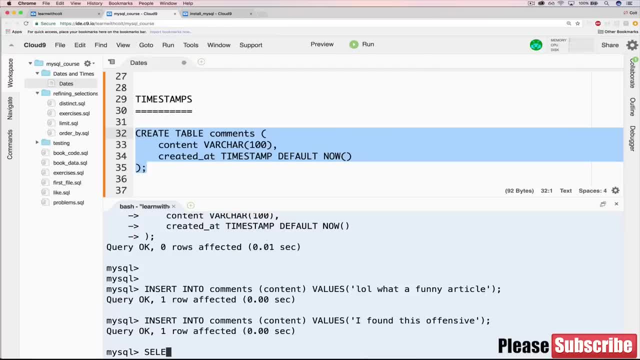 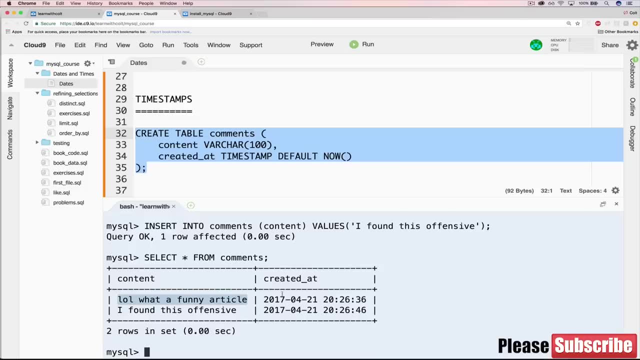 this offensive, Okay, So now if we do select star from comments, you can see: lol, what a funny article Created at. already filled in automatically Today's date, the time: 36 seconds. Compare that to. I found. 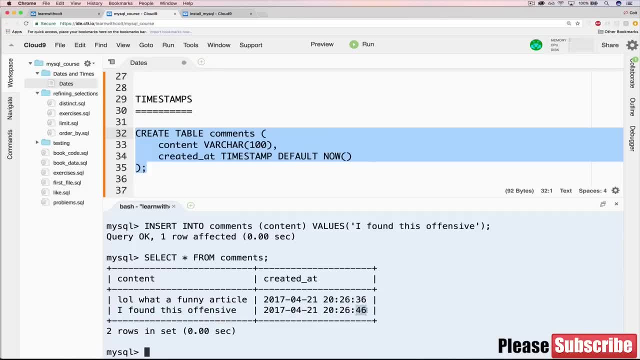 this offensive- Same date, same time- until we hit seconds. It was created 10 seconds later, So that's created at, And, of course, that's really useful. Um, I would show you how to sort them. However, they're already sorted here. 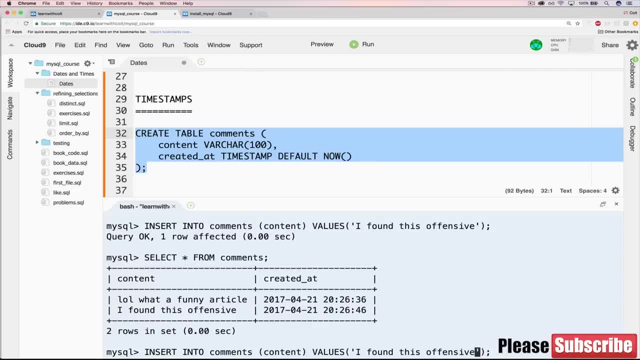 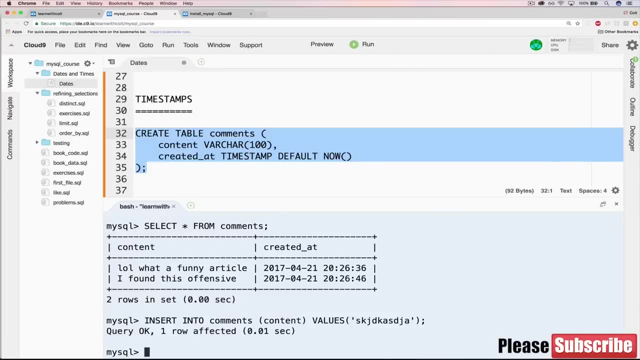 As you can see, because the order I'm putting in, or putting them in, is sorting them Um. but let me just try one more. Let's do just some gibberish, Select them all. Now we can do things like: 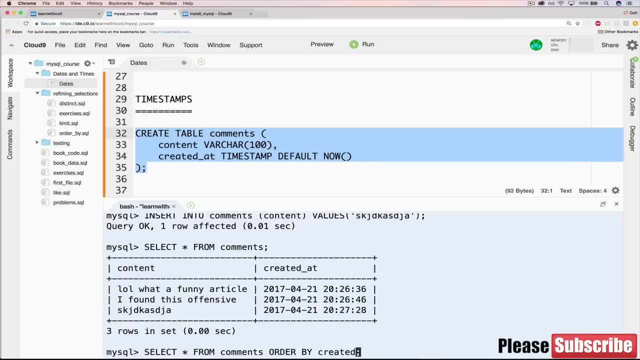 order by created at And that will order them basically the way they're ordered now. but we can reverse that. Change that to descending. Now we have the most recent comments up top, So that's created at using default now along with timestamp. But what if we? 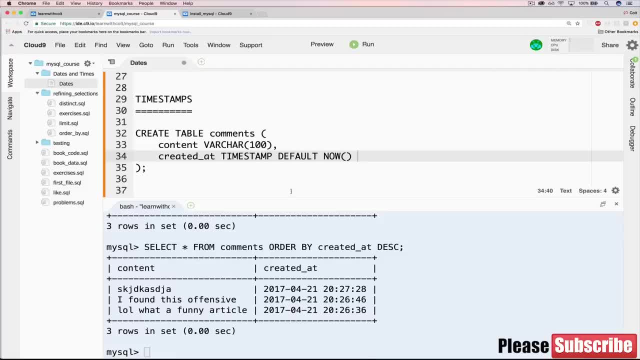 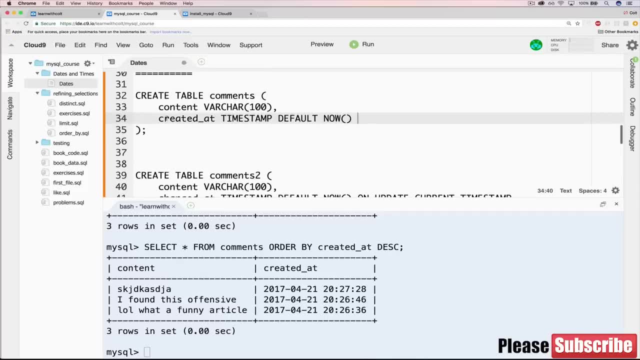 also wanted to store any time a field was changed. There's an easy way to do that as well: Just scroll down Magically hidden here. So I, instead of calling it created at, I made a new field called changed at, And the first part's the same. 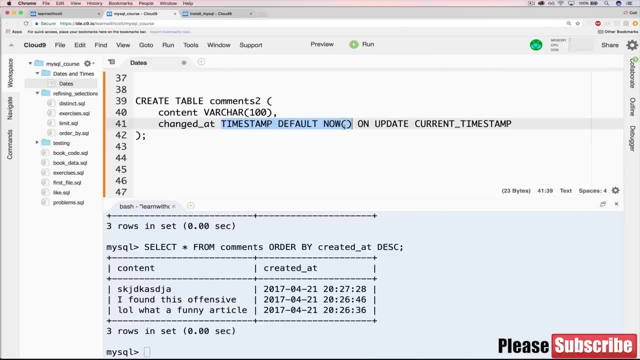 It's a timestamp and it sets a default value to be now, But then we get this on update, which we haven't seen before And, frankly, this is really the only time I ever use it. I don't know. I'm trying to think if I've ever used it in another. 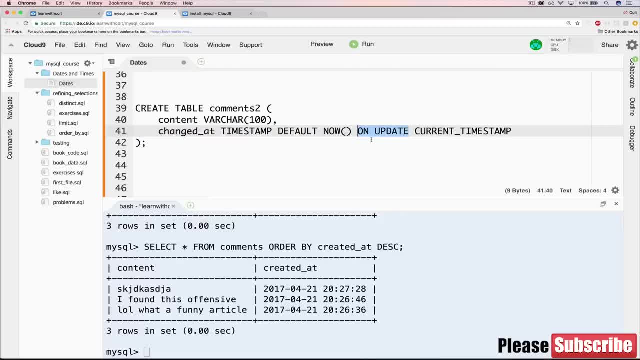 capacity Pretty much. this is the only way I've seen it used On update- current timestamp. So what this is saying is that when the row is changed, so if content is changed, then update changed at to be the current timestamp. So we could put something. 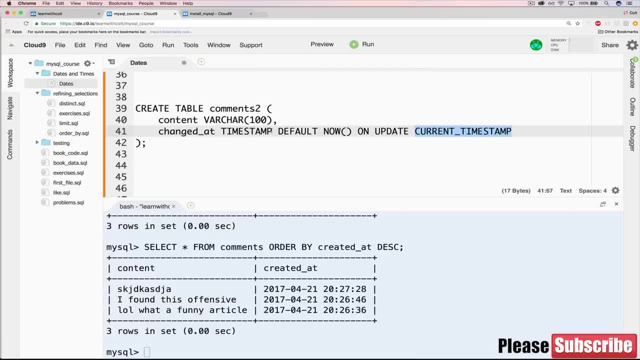 different here. We could put 3.. Although that's a problem because it's not a timestamp, But if we made this an int, I could do something ridiculous like this And every time that comments a row is updated, it will change that to be the number 3.. 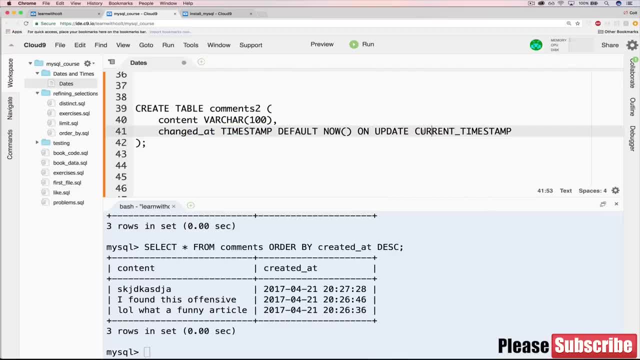 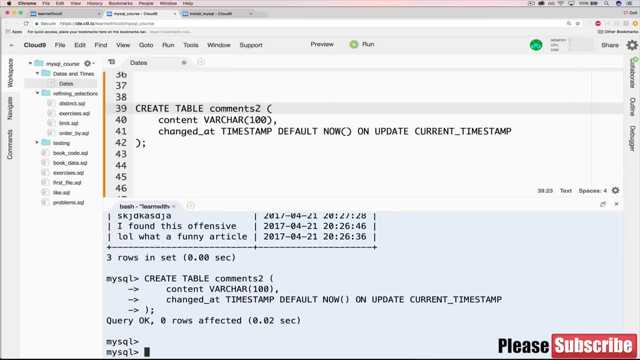 But there's no reason to do that whatsoever, so I won't. So if we run this, I called it comments2. by the way, I'm not running that out because I think it's original, but just so that you're aware. 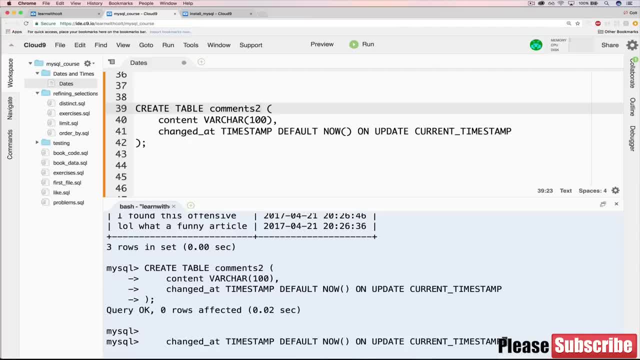 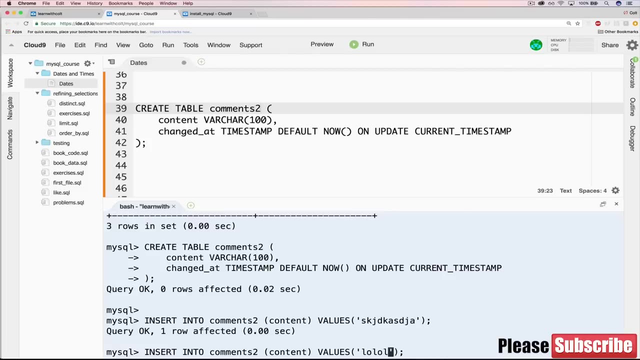 it's a different table If I now let me just use the same comments that I've already run And just change it to be insert into comments2.. So here's the first one, And our next one will be just lol, lol, lol. 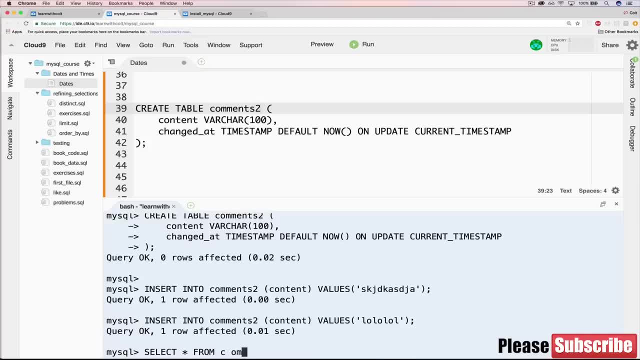 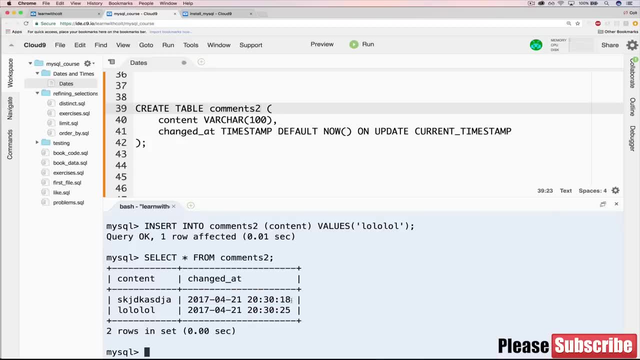 Okay, And now we do a select star from comments2.. You can see change that is filled in because we created them, And let's just do one more. This time will be: I like cats and dogs, just to please everybody, Unless you're a bird person. 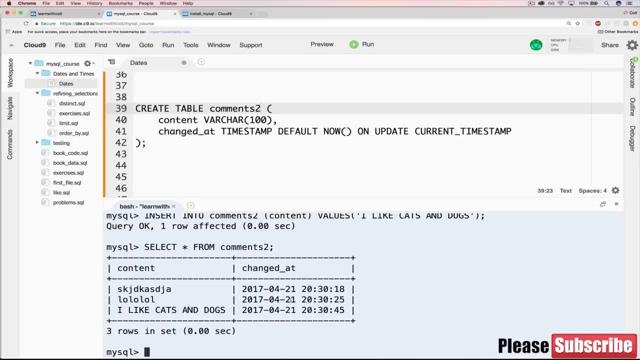 I guess, or you hate animals, So they're ordered by default because this is the order we added them in. There's no other way that they would be ordered. But let's try updating one, Okay. So let's update this gibberish here to say: 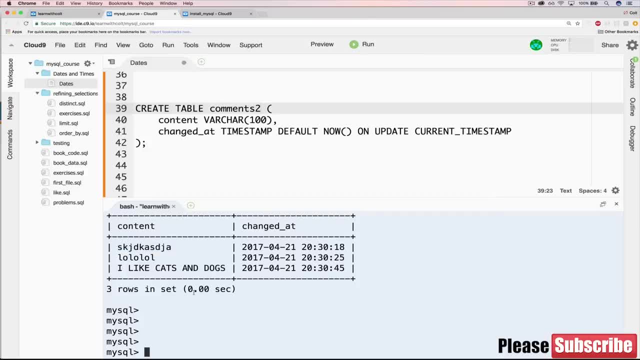 something else. It's been a while since we've done an update, but hopefully you remember. So we're going to want to update comments2. set content equal to- and let's say, this is not gibberish, Something like that, And then 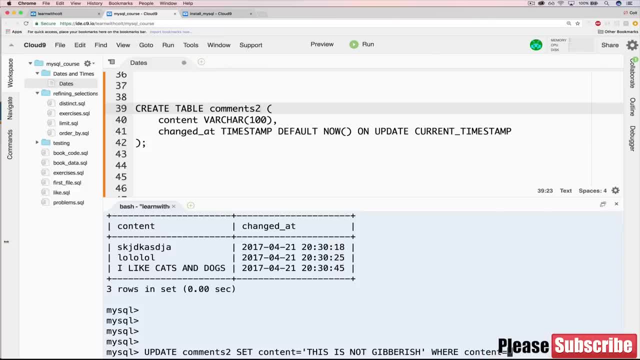 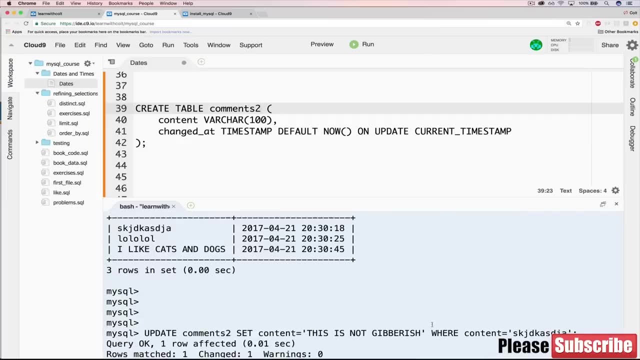 we need to specify where content is currently, this mess of gibberish. Okay, So if I update that notice what we had before: 20-30-18.. The date's not going to change: 20-30-18.. 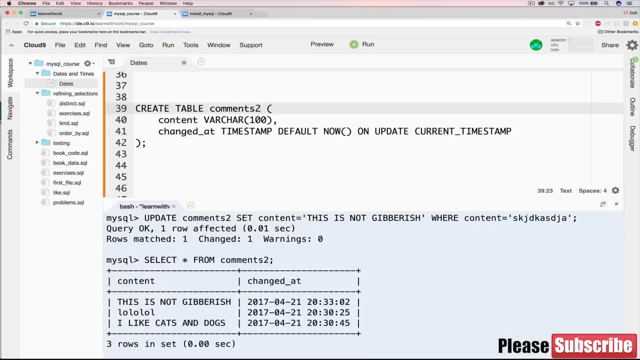 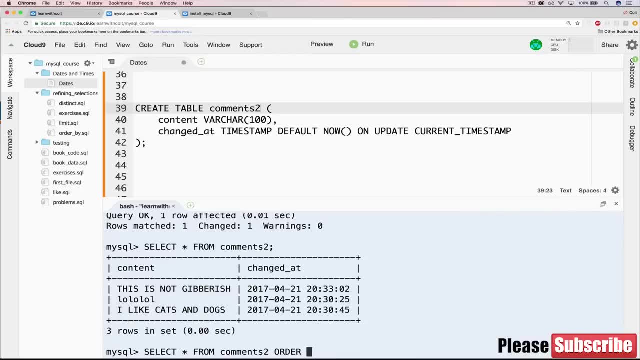 Now, if I do a select star, it's changed to 20-33-02.. And so now, if we order things by what do we call it? Change dat. You'll see we now have a new order. So that's really important. 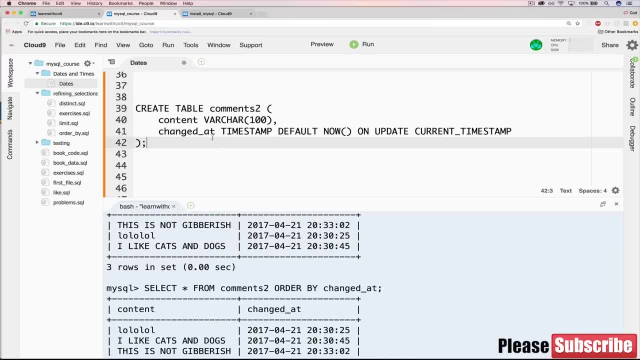 to take note of is that if you want to not only track when something was created, but when it was updated, you can use this setup here. So we have timestamp default now On update. oh, one thing I didn't talk about: Current. 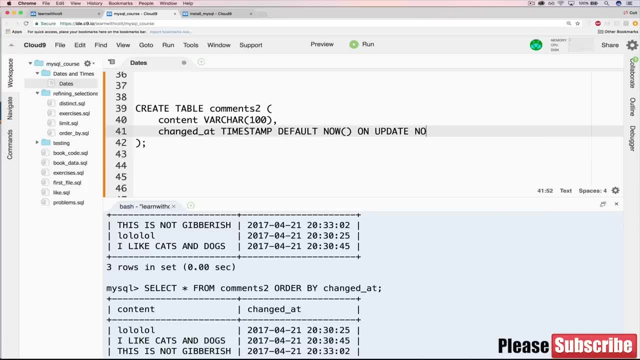 timestamp You could also put now here. The reason I didn't is just to show you you can also use current timestamp. It's just another shortcut I prefer to use now, just because it's, like I said, a couple times, short, simple, easy to remember. 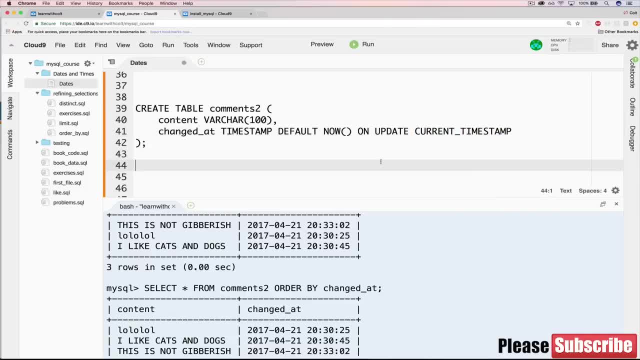 But current timestamp does the exact same thing in this case. Okay, So this is something, a bit of a recipe that you'll probably return to. It's worth knowing You'll see me use it as we go in this course and some of the other. 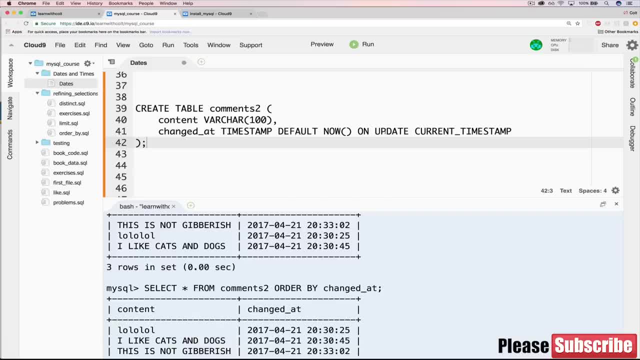 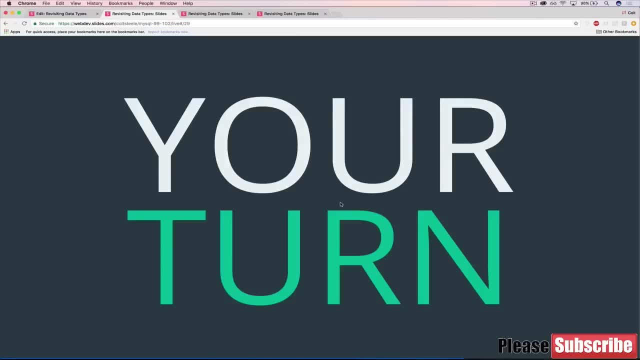 schemas that we create as things get more complex. It's important, It's useful, to store that metadata about when things are created or when they're updated. Okay, We're done. Okay, So we're at the end of this section And, as always, it's your turn. 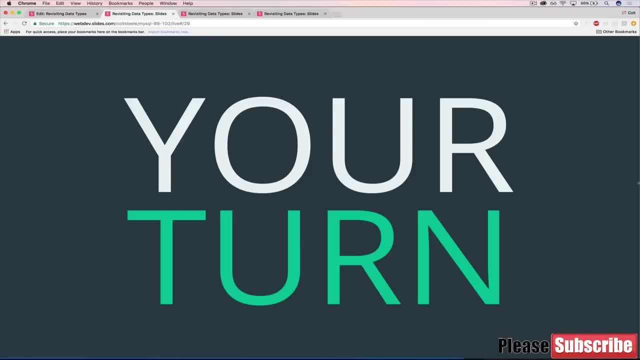 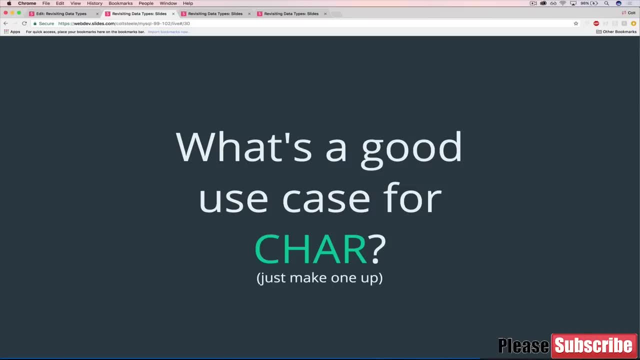 to put it into practice, As you can see by these giant letters. So we've got a couple of problems here that cover basically everything we talked about- Well, not everything, but all the big things we talked about in this section, All about data types. 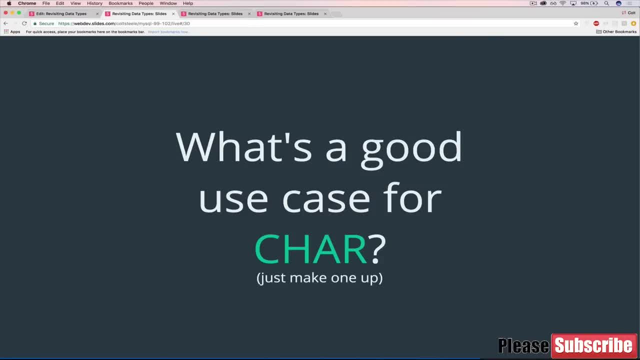 So strings, text data types, numeric data types and then date and time information and ways of working with those dates with some of the more common date functions. So there's a couple of exercises here. Some of them involve writing code, Some of them are fill in. 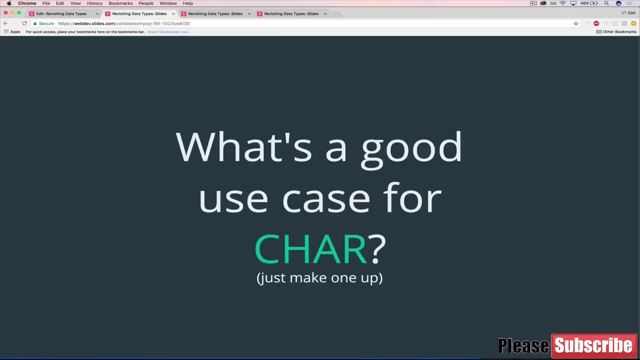 the blanks. Some of them are just- I don't know what you would call this Free response Like this one here. So let's get started And then in the next video we'll have a solution. So this one what's a good use. 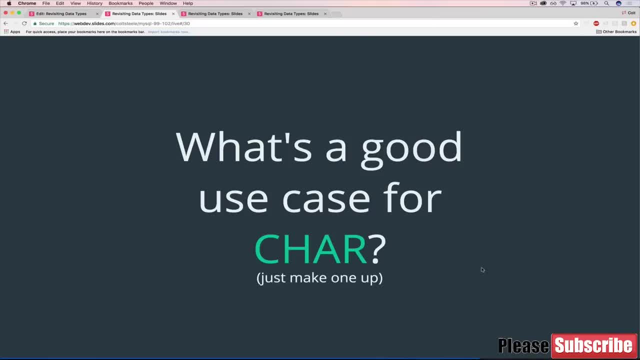 case for char Or chair. No, not chair, Char Or car- That data type. So when would you use that instead of or in lieu of var char? So you can use one of the things that we talked about or come up with your own. 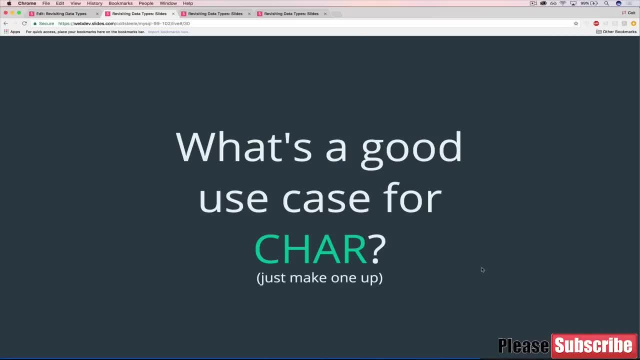 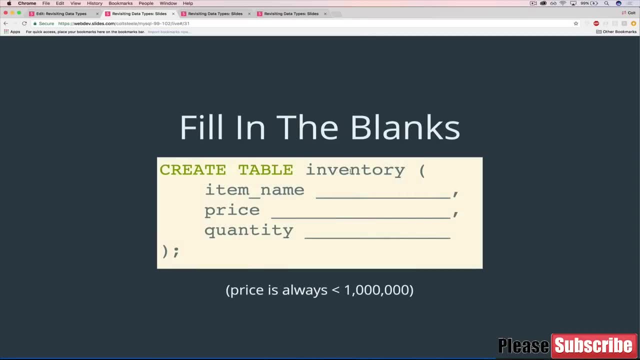 You don't have to write it down, Just come up with something Next up, fill in the blanks here. So we've got a table that I'm creating called inventory or inventories or whatever, Some sort of something that we're storing. 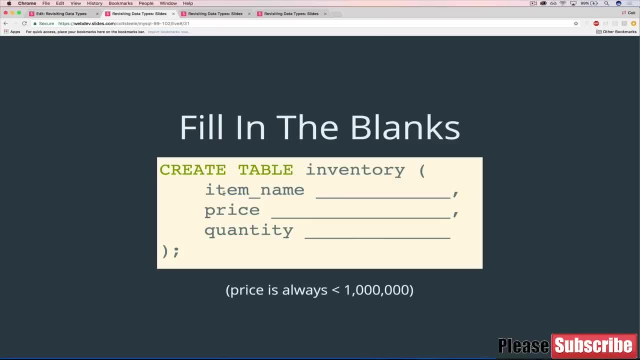 Books or toys. We've got an item name. What data type should that be? There's not necessarily one, only one workable answer, but there's one better answer: Price. So what data type should price be, And not just the type of? 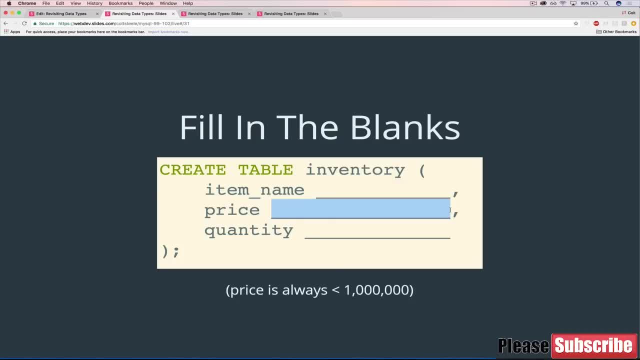 or not just the name of the data type, but what are you going to put in those parentheses? And as a note, all of our prices are less than one million dollars, Not equal to one million dollars. just to be clear. They're less than. 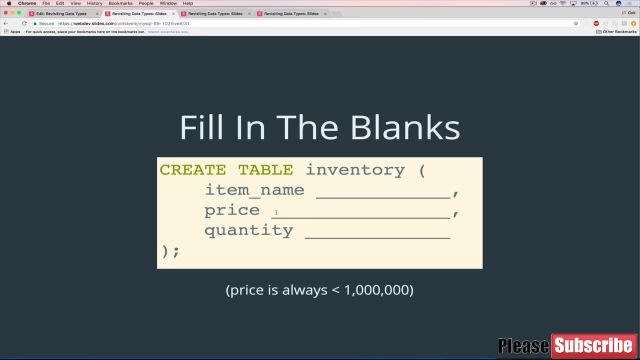 one million. So how would we represent that with our data type? And then quantity, That's a number as well. What data type makes the most sense there? Okay, Then moving on, What's the difference between date, time and time stamp? 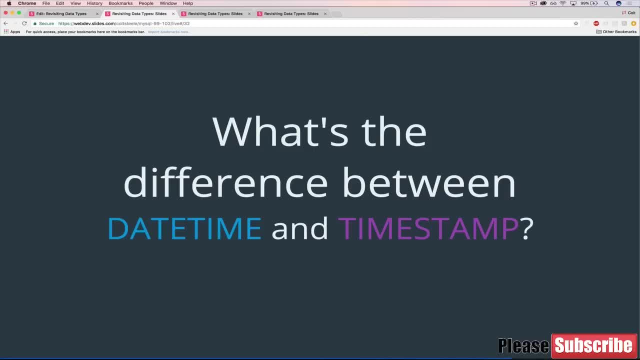 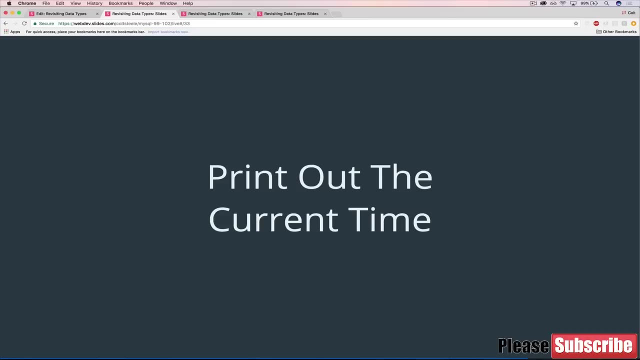 There's not just one difference, but one versus the other. How are they different? We talked about it, We looked at the documentation for both of them, So hopefully it's not too hard. Next up in Cloud9, print out the current time. 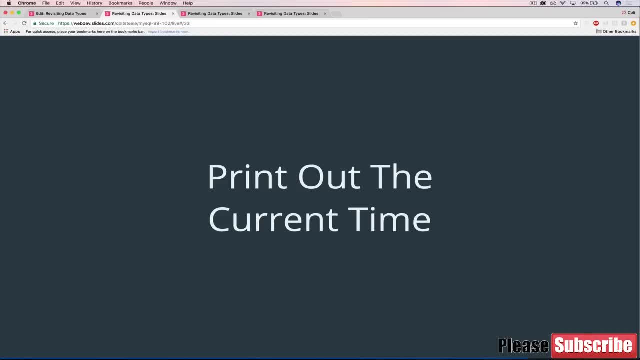 using MySQL, So just the time. Then the next question is to print out the current date but not the time, So just the date. And then, once you've done that, print out the current day of the week, the number of the day of the week, 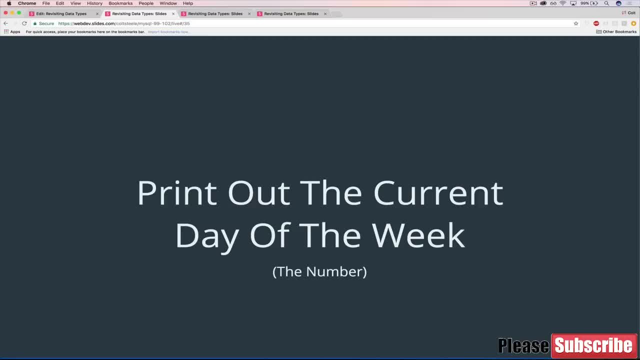 So if it's a Saturday, it should be 7.. If it's a Friday, 6 and so on. So just print that out And then do the same thing. Print out the current day of the week, But this time it should be the name of the day of the week. 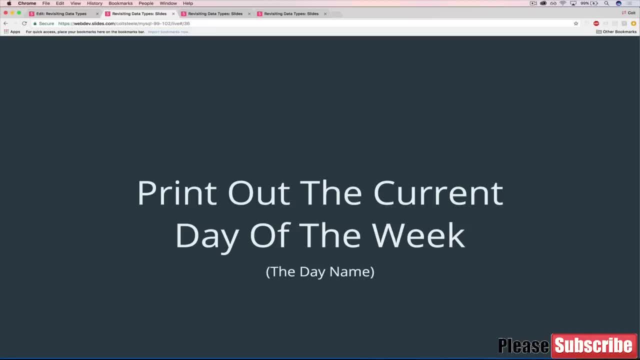 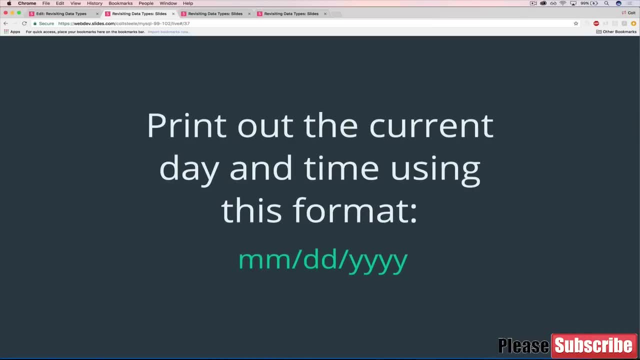 Like Monday or Tuesday, So the English name of the day of the week for today. Whenever you're running this, print out the day of the week Next up. print out the current day and time using this format. So month, month slash, day, day slash. 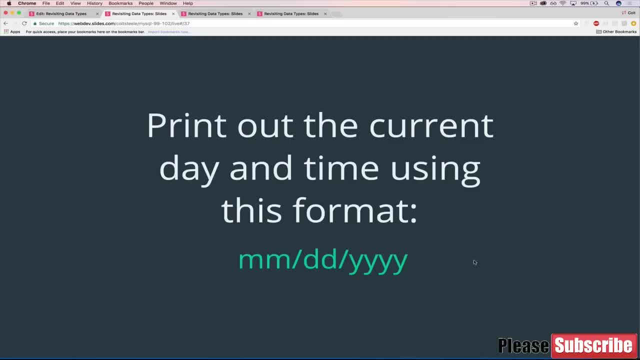 four digits for the year And then, once you've done that, we have another one. Print out the current day and time using this format, which I wasn't sure how to actually boil this down to a nice little formula like we have here, So I just gave you two. 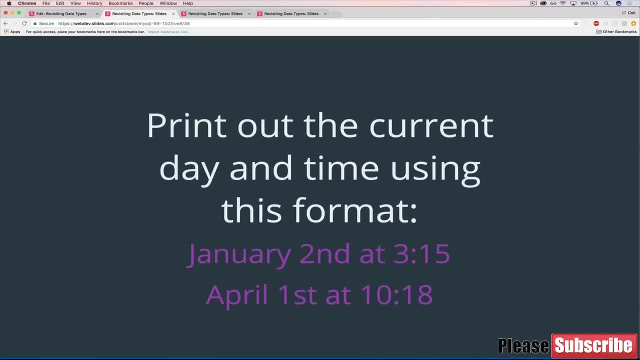 examples. So we have the full month name: January or April. Then we have this, which there's a name for it. I think it's anglicized. what is it Anglicized? digits or something. It's in the documentation. We didn't cover this. You'll have to dig around. 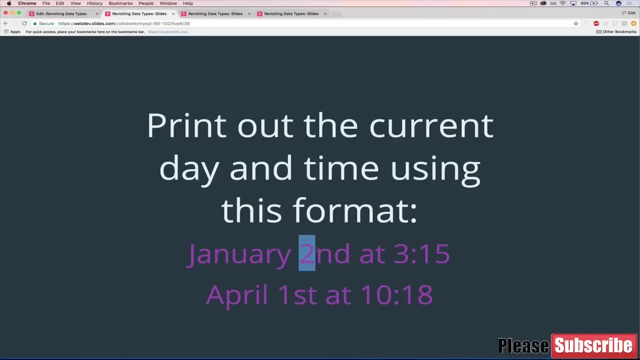 to figure out how you format it this way, But with the day of the month, like two or one, But instead of just the number. we want this anglicized version. So second, first, third, tenth and so on, And then 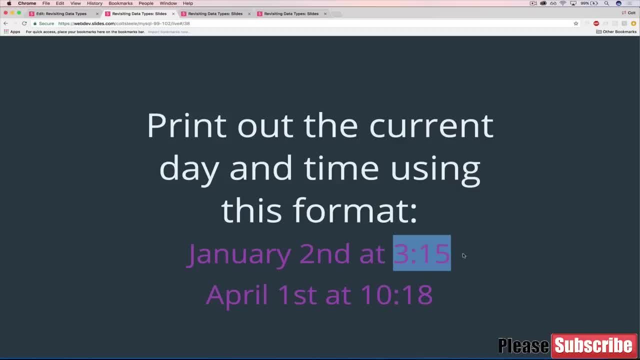 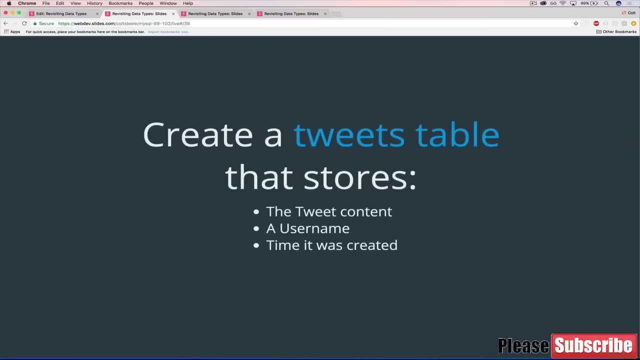 at, and then the time, And for the time, we just want hour colon minutes. Okay, After you've done that, we have one final thing: Create a tweets table, And the tweets table should store the content of a tweet. So that's going to be text. 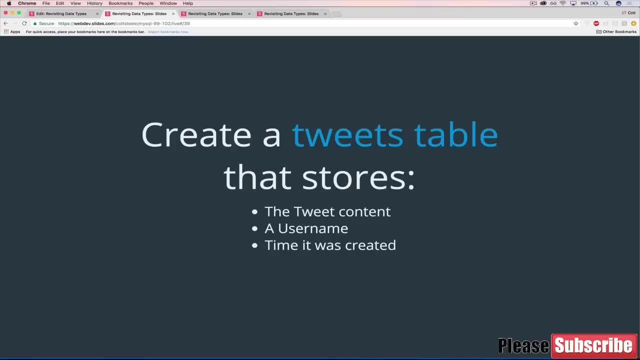 And I believe, what is it? 140 characters And then a username, And we don't need a character limit for that. Let's I don't know. let's say 20 characters, But that's not that important. And then we also want to store. 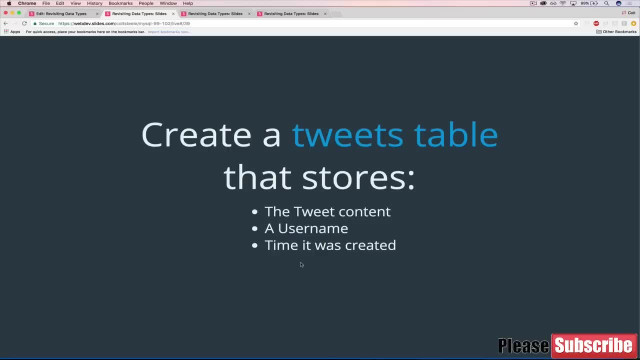 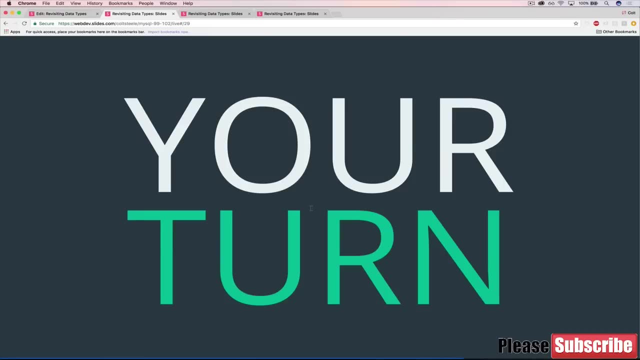 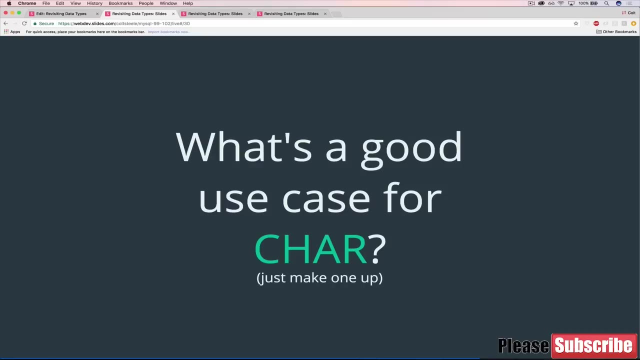 the time the tweet was created. Okay. When you've done that, pat yourself on the back, Okay. So this is the solution video to our data types problem. set First one here. What's a good use case for char? So there's not a ton of times that I end up. 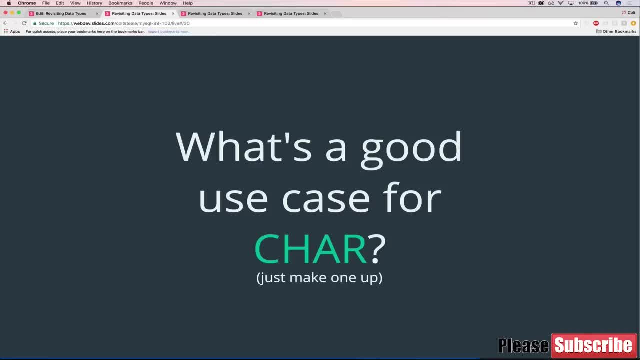 using them. but remember they are fixed length so we have to specify exactly the length of the char that we want for that column. So we often will use it for text that we know 100% has a fixed length. So the one that I've used a couple times is: 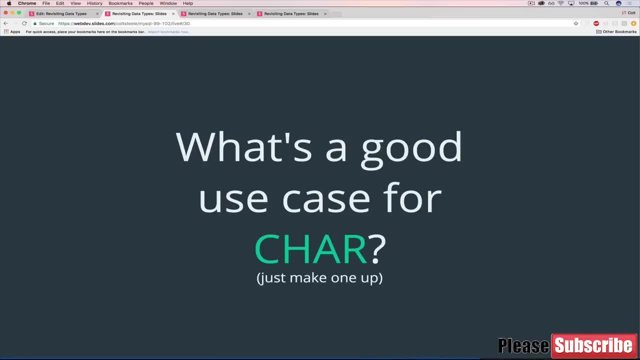 state abbreviations. If you're doing sex, like M or F, or perhaps you're working on a project where I don't know, let's say you're working with companies and you want an abbreviated name for every company. that's only 5 characters. 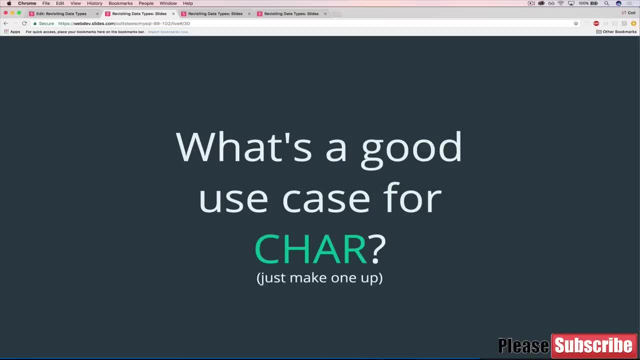 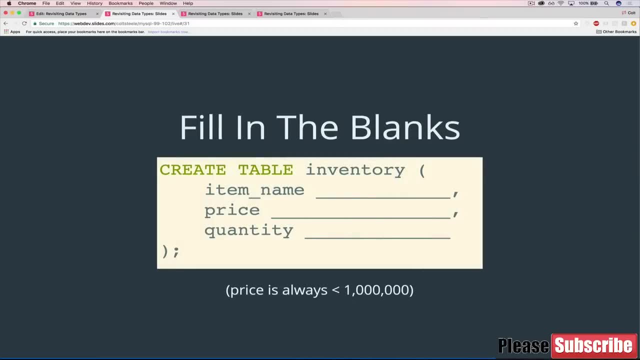 or 4 characters long. Then you could use char as well. Hopefully you came up with something better than me, Something new and original. Next up, fill in the blanks of this schema. Okay, so there's a couple things to talk about. 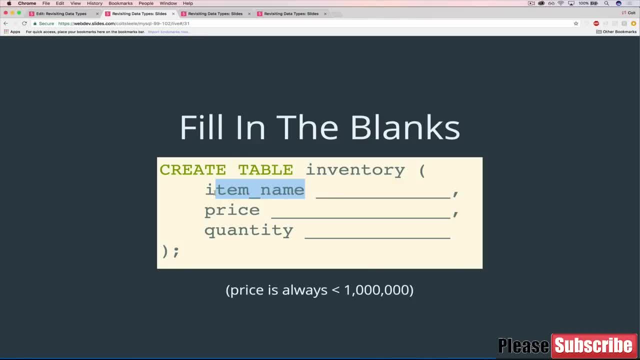 Item name is text. It's going to be something like I don't know, cabbage patch doll or baseball hat, And that should be a var char. most likely You could get away with using a char, but there's no reason to do that because it's not fixed length. 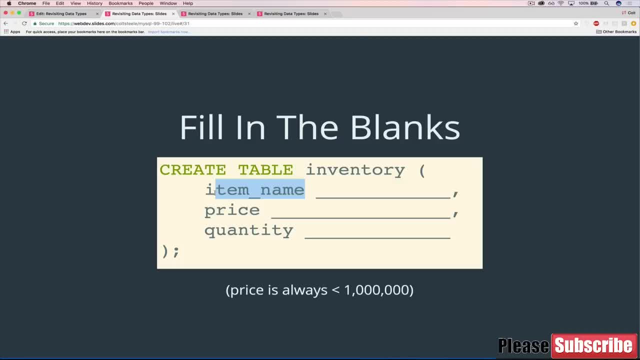 So it makes more sense to do var, char And then quantity. I'll skip price for a moment. Quantity makes sense to be an integer. We are never going to have partial items in stock. We're not going to have 2.5. 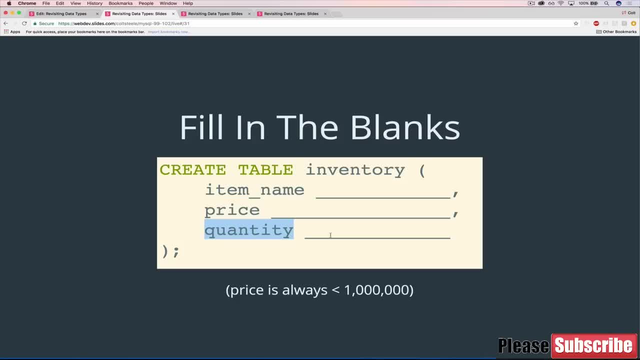 cabbage patch dolls. hopefully, Unless there is some sort of massacre with the cabbage patch dolls and the chainsaw, We're hopefully only going to have whole numbers of them, So we'll use int. But price is a little trickier And so I added this note: Price is always. 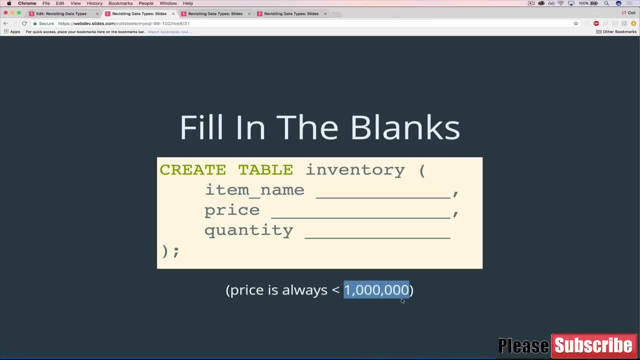 less than 1 million dollars? Okay, but price is not usually, or not exclusively, a whole number. We want to allow for cents, So we're going to want to use a decimal. Now, you could use a float or a double, but, as we discussed, decimal is. 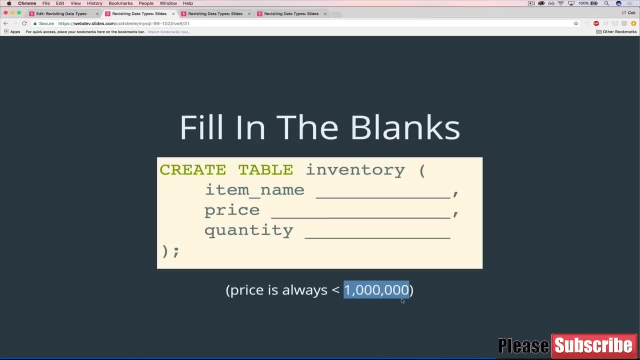 better for monetary stuff because it's more precise. You don't have to worry about losing precision as you get into longer numbers. Okay, so then the question is: what do we put here? It's not just decimal on its own. We don't. 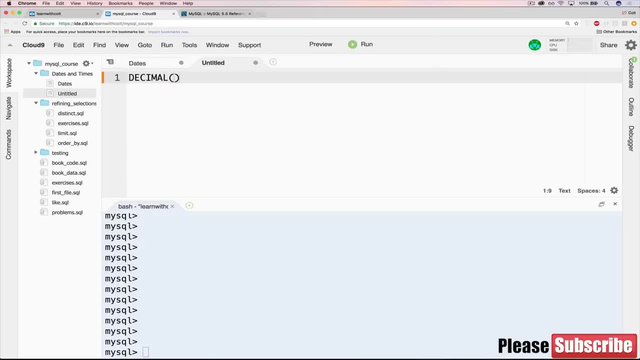 just do this. We have two numbers we pass in, And those two numbers- if you can remember the names, I believe the first one is precision and the second one is scale. Don't quote me on that, though, But basically it's a total number. 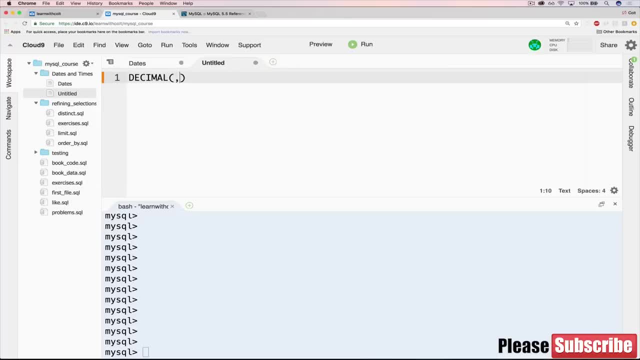 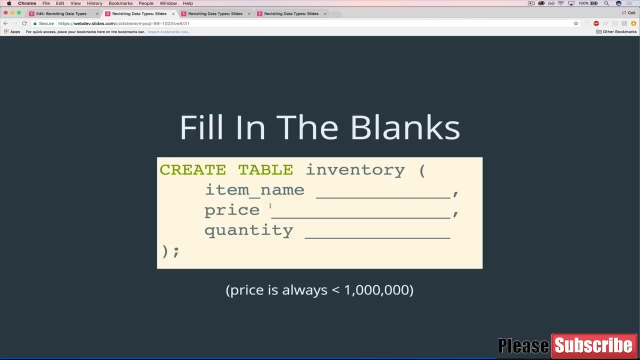 of digits, followed by the number of digits after the decimal. So we can start with the number of digits after the decimal, which, when you're working with price or monetary information, it's pretty much always 2.. So then the question becomes how? 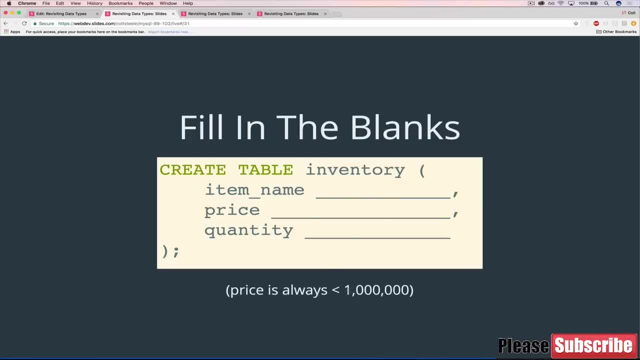 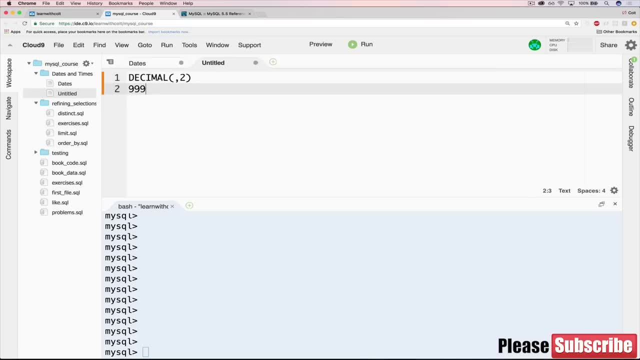 many total digits do we need? And if I said it's always less than, excuse me, it's always less than 1 million. that means that our highest price we could have is 999,999.99.. So if that's the maximum, 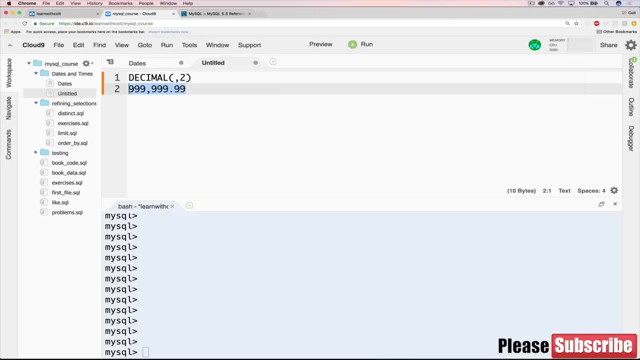 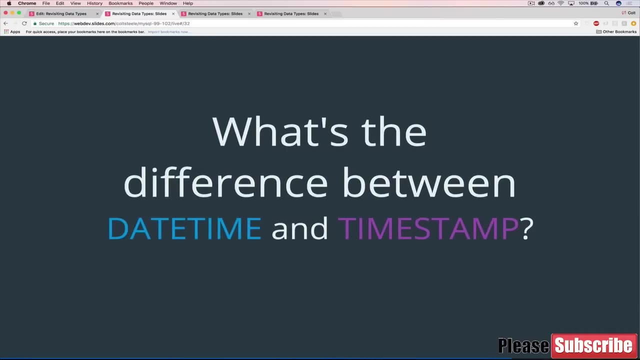 price, then all we need to do is count out the total number of digits. So that is 3678.. And that's our answer: Decimal 8, comma 2.. Next up, what's the difference between date, time and timestamp? 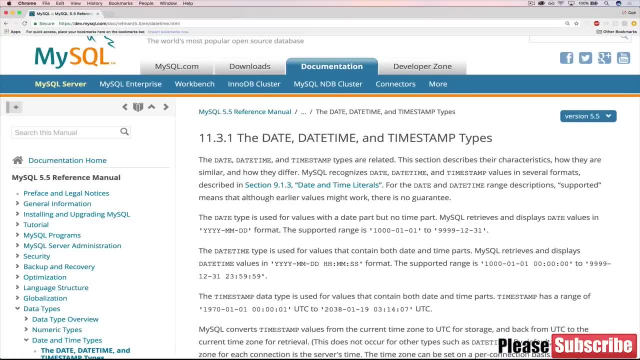 So I have the documentation open for date, date, time and timestamp, And the first thing I'll say is that there's a couple of differences. There are a few technical differences as far as how they're stored and the ranges that they support. 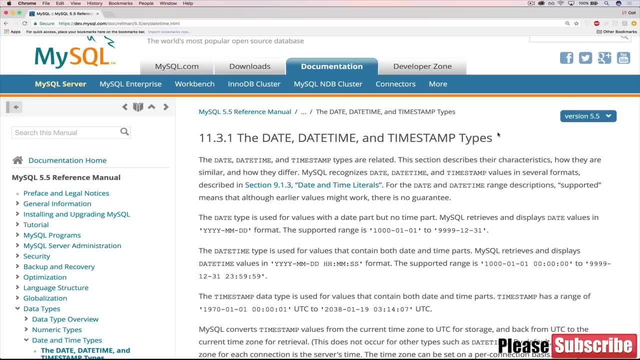 And then there's a big difference into how they're put into use most of the time. So both of them, let's start off. they both store date and time information, So they store the date and then the time. However, there's a big difference in. 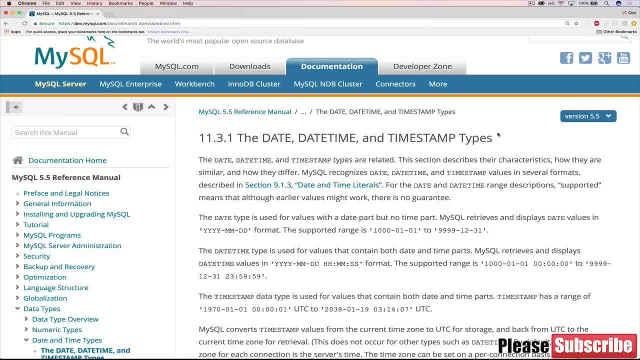 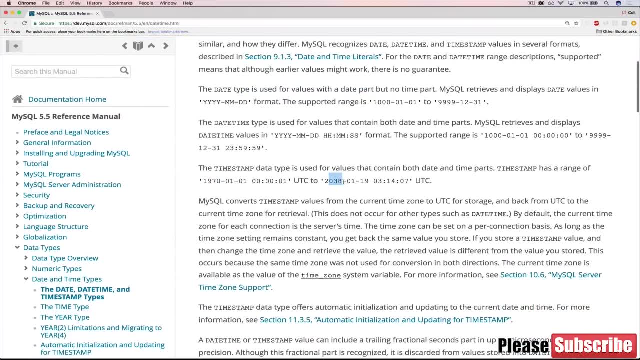 the range that they support. So timestamps have a much smaller range. If you remember, we went over this. Where is that? Timestamp has a range from 1970 to 2038.. Versus date time goes from 1000, year 1000, up to year 9999. 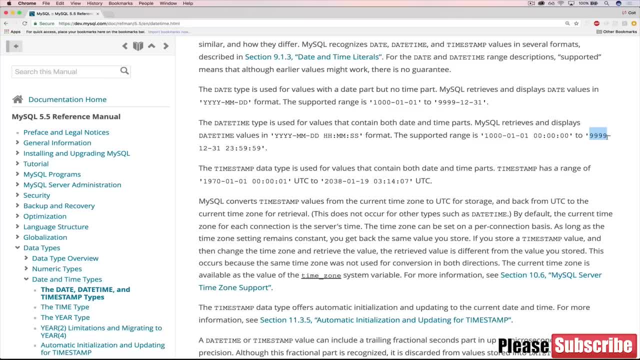 So that's one significant difference. The other is the size or the memory they take up. A date time is roughly twice as large as timestamp, Which brings us to the final difference, which is how they're actually put into practice, And typically, 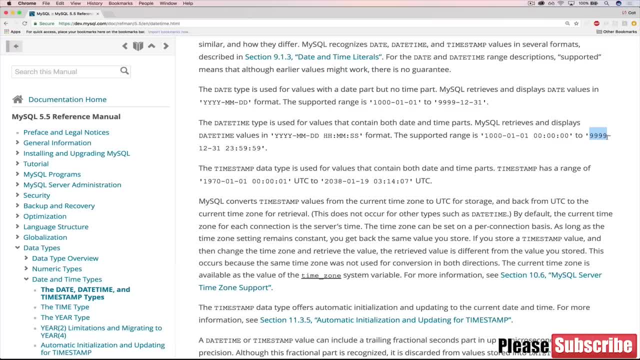 timestamps are used- at least in my experience- exclusively when we are trying to add metadata about when something is created or updated to a table. Otherwise, I use date time. Now, that doesn't mean that you can't use timestamp. If you wanted to use timestamp to store, 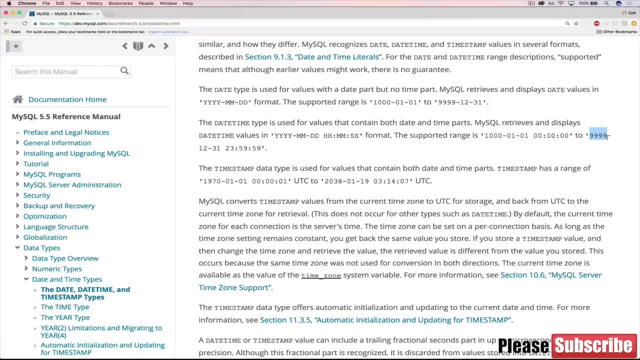 birthdays. you could, but you could run into problems if you have people who are born before 1970.. So again, the key differences really boil down to the ranges they support and then how much memory they take up. Okay, moving on. 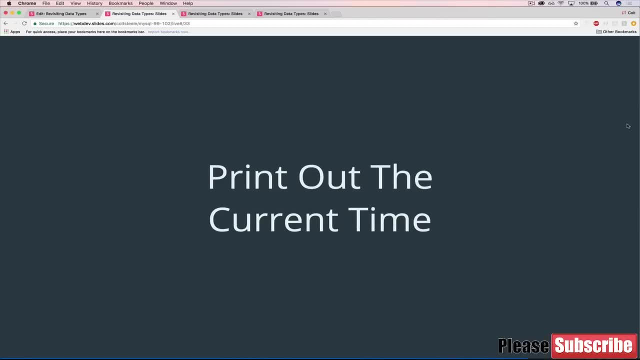 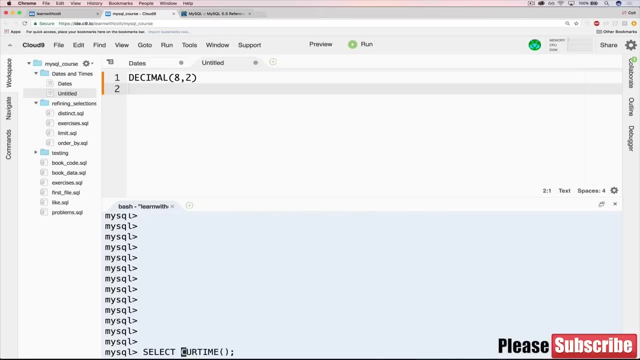 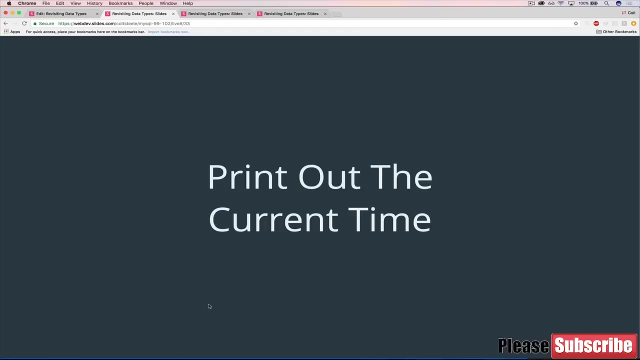 Print out the current time. Finally, some code So to print out the current time. it's just a matter of cur time And we need to select that. There we go: 160813.. Yours, of course, will differ most likely. 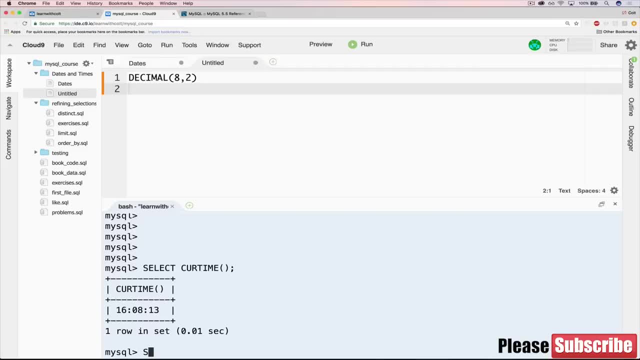 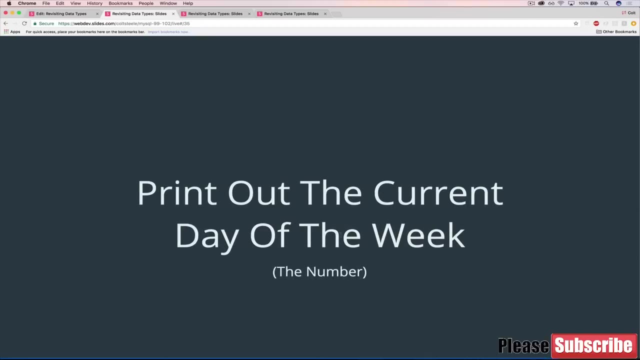 Print out the current date but not the time, So that one we want to do cur date, As you can see, April 22, 2017.. Still my birthday. Print out the current day of the week. Okay, so this one's a little bit different. 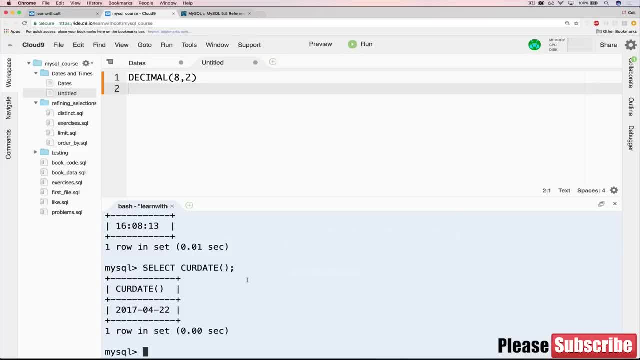 There's a couple ways of achieving this. The first one is to use select day of week, and then we could either give it the date cur date, or we could use now. So today is a Saturday, so it gives us 7.. 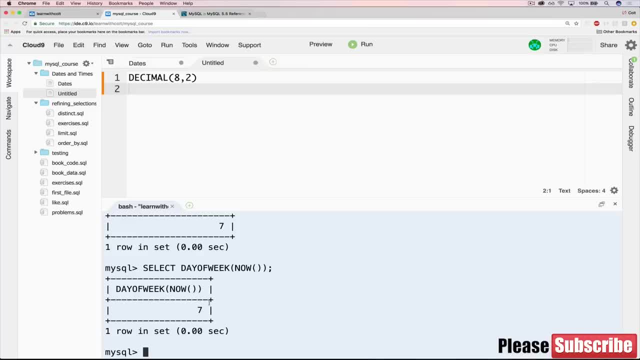 Just to show you, I can replace this with now, which is a date time, and I also get 7.. But there's another way we could do this, which is to use date format. And if we go to the documentation here, 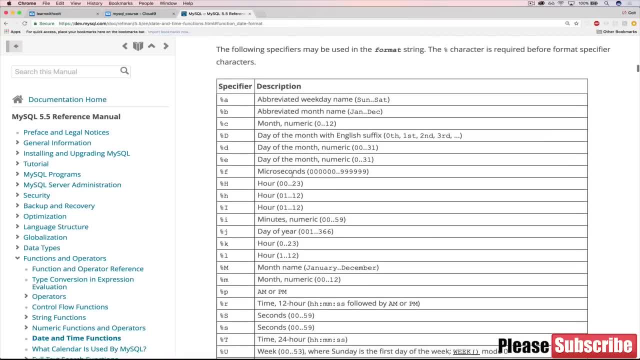 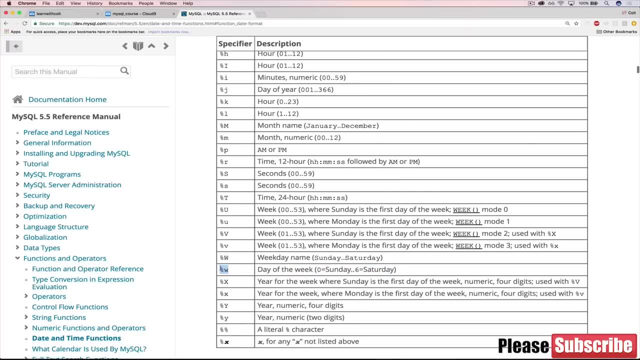 and we find this date format if we scroll down somewhere on: here is day of the week. Where is that? Here we go, Day of the week. percent w lowercase w. So we could use that Do select date format. 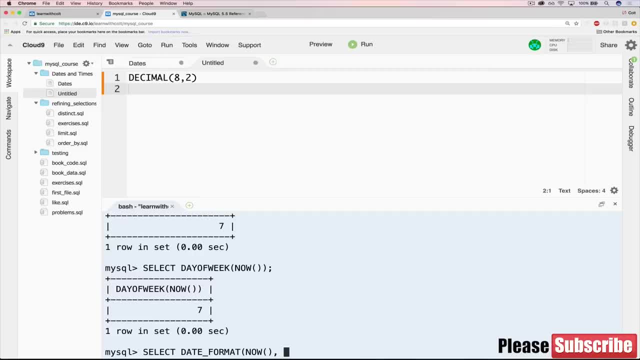 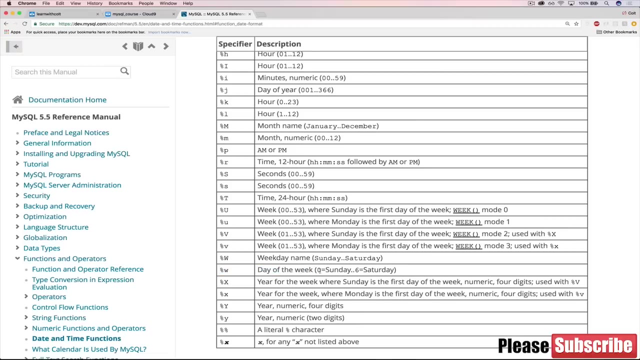 now, or cur date comma, and the string we want is just percent, lowercase w, And actually I didn't know this until now. there is a difference. It's kind of fascinating. If we read this closely, it says day of the week. 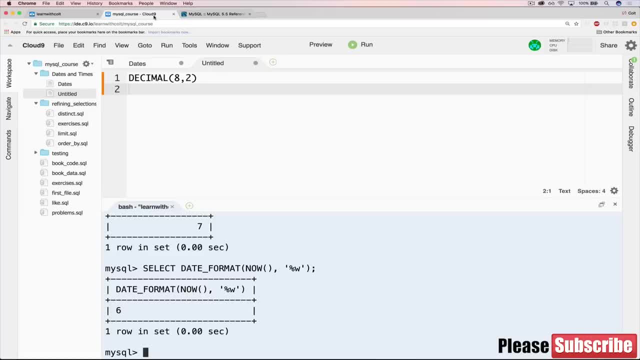 zero is Sunday and six is Saturday, So these are not equivalent. actually, Day of the week, Sunday is one rather than zero And Saturday is seven. So I guess if we wanted these to be equivalent we would need to do a plus one. 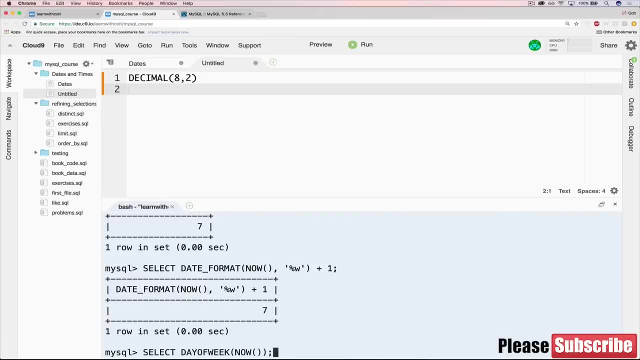 And shift everything by one, or shift everything down one if we're using the previous Interesting. No idea why that's the case, but it is what it is. So the next thing is to print out the current day of the week, but I want 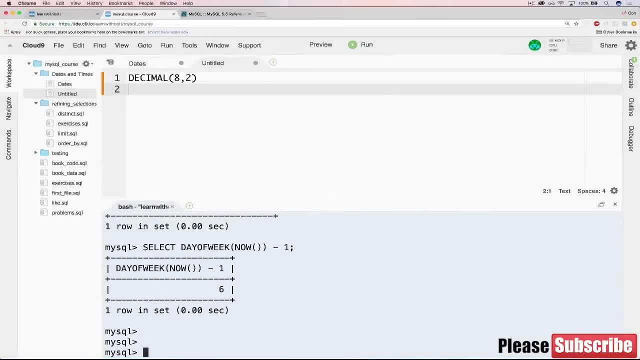 the date name. Day name: Monday, Tuesday, Wednesday and so on. I wouldn't expect you to remember this, but there is a day name that we can use, Like that, Select day name, Or we can do our format date, our date format. 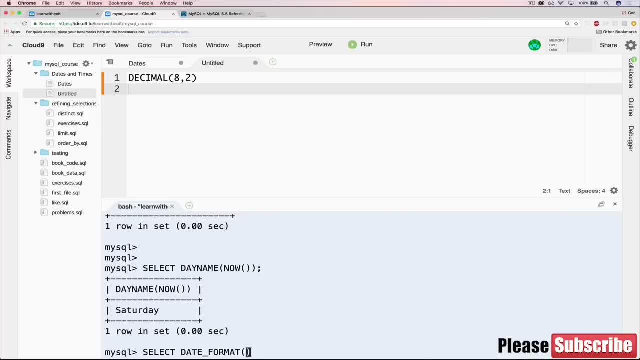 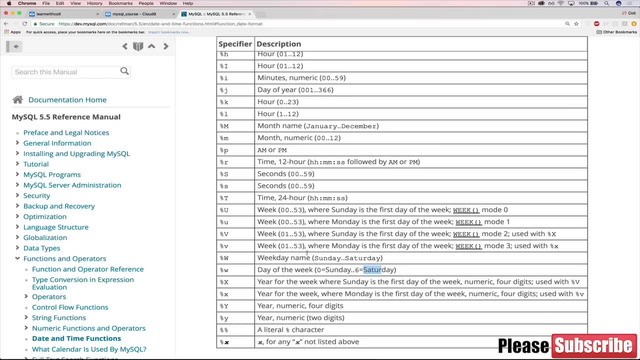 I always mix up the order there, but it's date underscore format for now, And then we just have to figure out how we get the day of the week name. So if we go to the docs, it's right above Weekday name, Sunday. 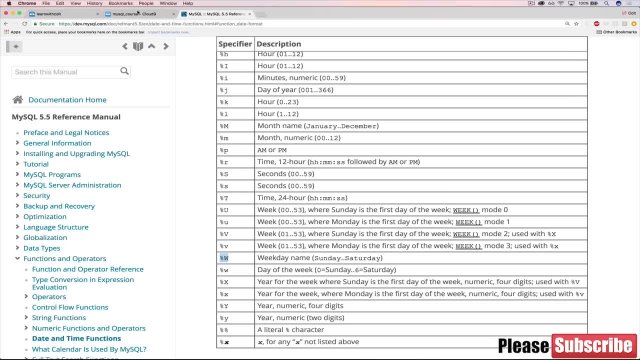 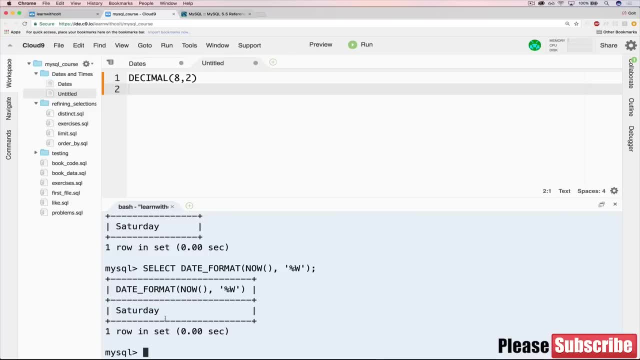 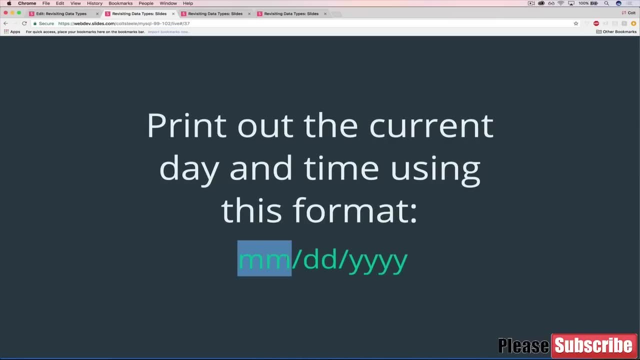 to Saturday: percent uppercase W. So if we switch back, just change it to an uppercase W. now we get Saturday, Okay, Next up. print out the current date and time using this format: Month month slash day, day slash year, year, year, year, year. 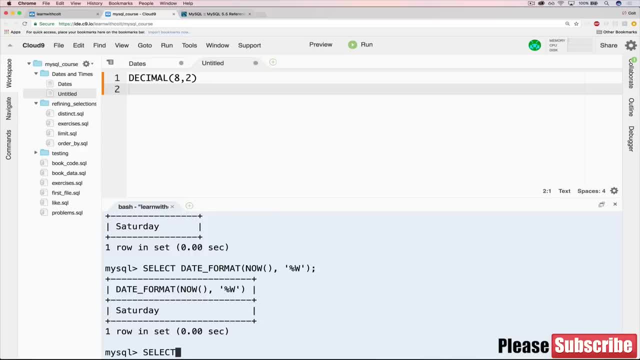 Okay, So we'll need to use date format And we can just use cur date, or we can use now. I like to use now typically, But we're not actually using the time information, so why don't we just use cur date in this case, just to show. 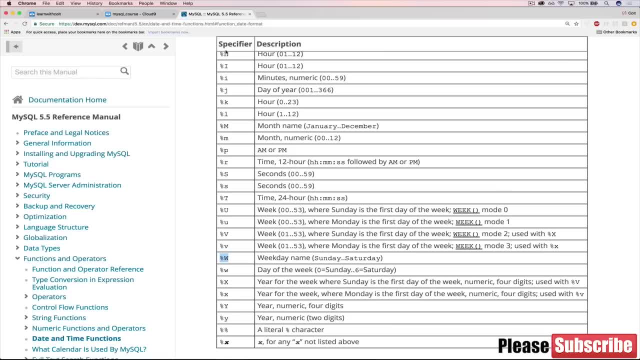 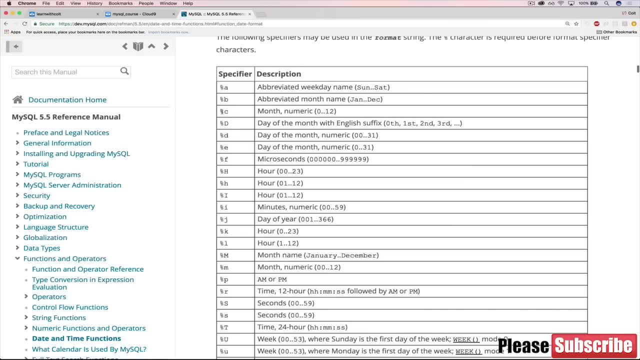 you, we can, And then the way we want to format it. if we go to the docs, we want first of all what's the month? So we want month numeric, which is percent. oh no, that's not what we want. What we want is: 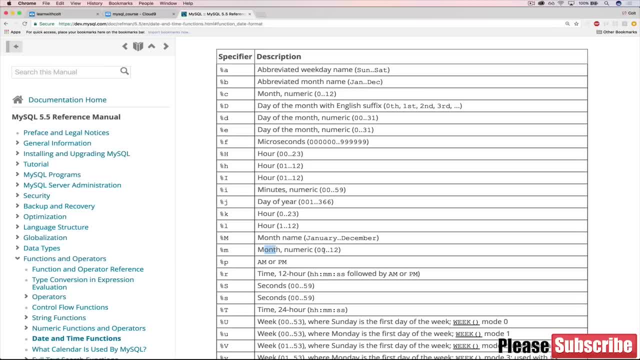 down here This Month, numeric 0 to 12. So we get m lowercase m percent, lowercase m slash, and then we want day of the month, numeric 00 to 31,, because we want those two digits always. 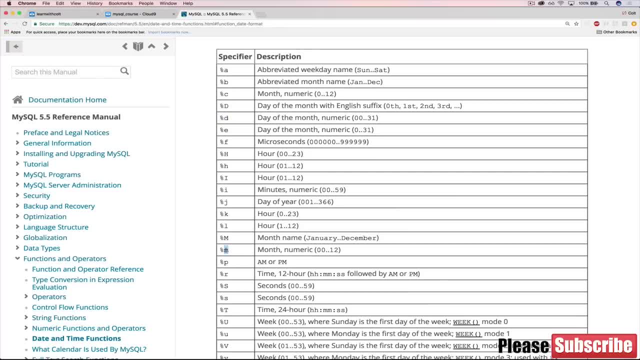 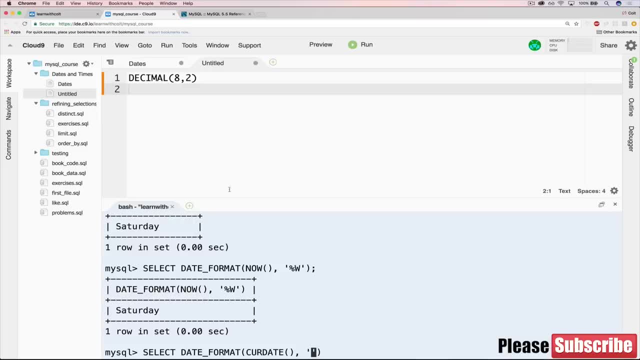 So that's lowercase d. So we have lowercase m slash lowercase d, and then for year we want four digits, So that's uppercase y. So let's try that: Percent lowercase m slash percent lowercase d. 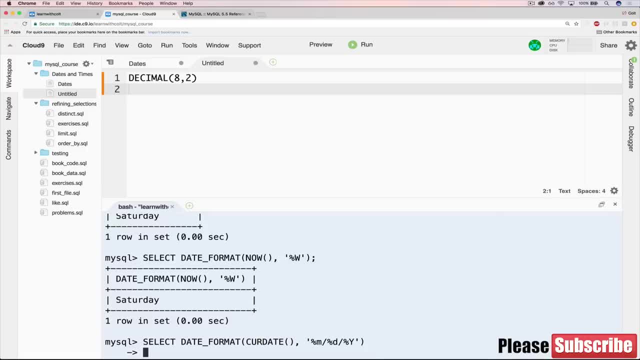 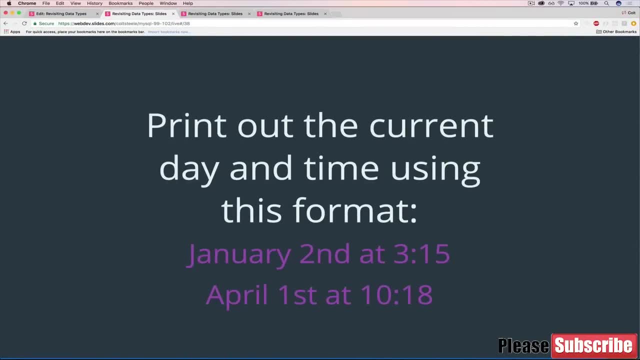 slash percent, uppercase y: Oh, semicolon, There we go, And that works. Next up: print out the current day and time using this format. It's a bit different. We want the month name and then the anglicized day. 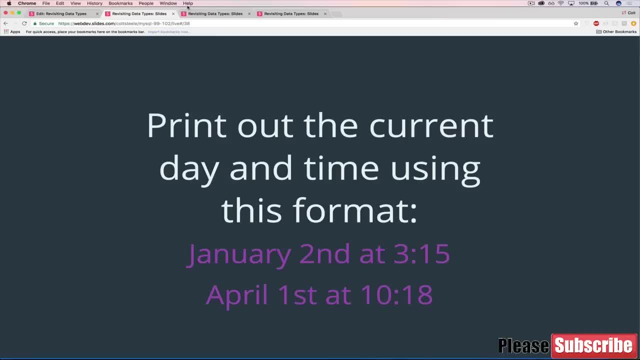 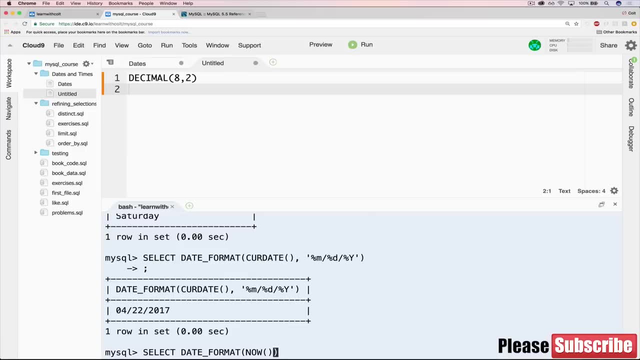 at, and then hours and minutes. So let's start off with what we know. We're going to need to use date format, and we need to use now, because we need date and time rather than cur date, which gives us just the date. 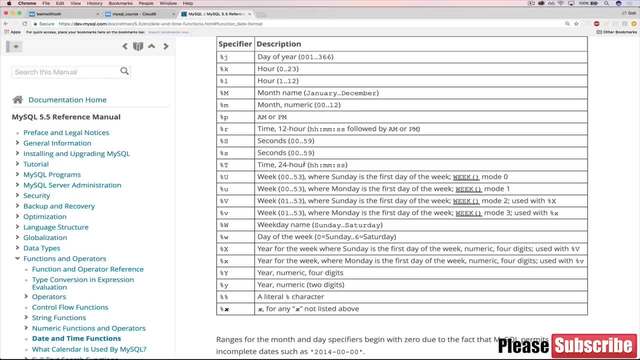 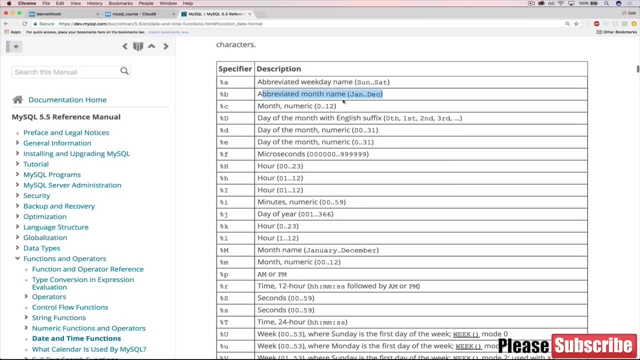 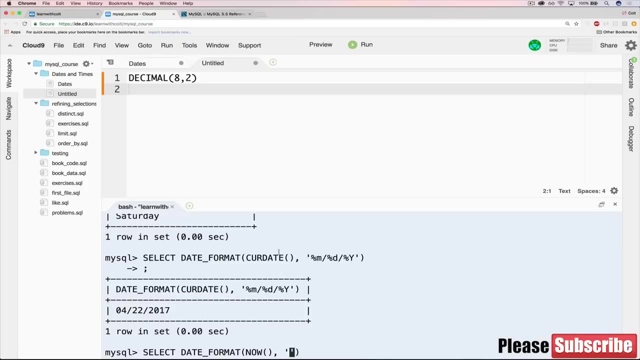 Then our format string. First thing we want is the month name, which is right. where are you? This is abbreviated month name. Here we go. Month name uppercase m. So we want uppercase m space. and then the anglicized version. 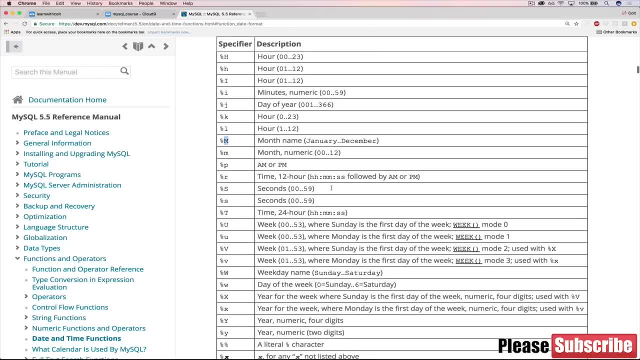 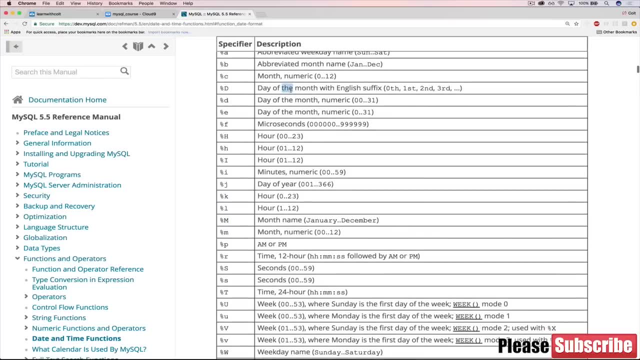 of the day. And where is that? Here we go. Day of the month with English suffix. That's what I was trying to say. So it's uppercase d. Okay, Let's just see if that works. to start, There we go. April 22nd. 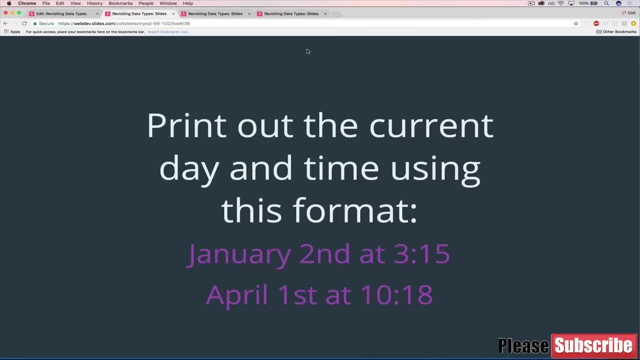 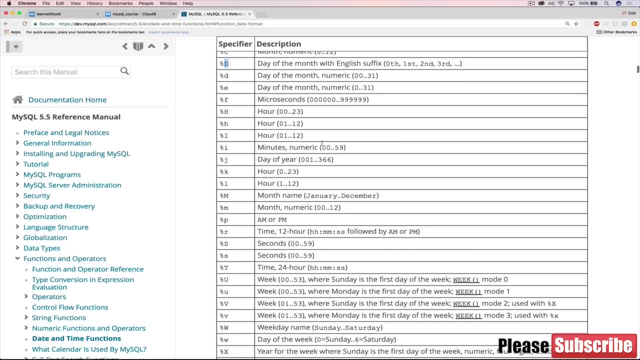 Followed by at. No years necessary, so at. and then hours and minutes. So again hours. we have lowercase h if we want. I guess I didn't specify if we wanted 24 hour time or 12 hours, so 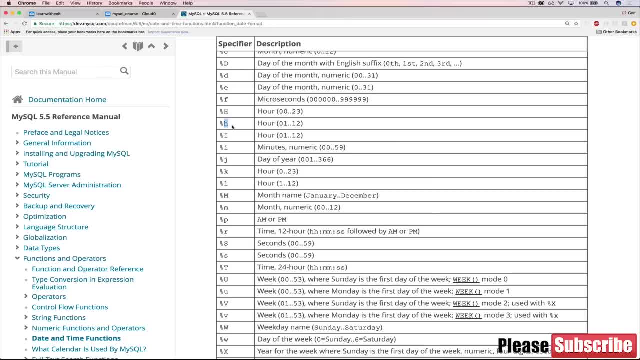 either of these will work. I'm just going to do lowercase h colon and then for minutes it's lowercase. well, let's see, i is going to give us. there we go, That will work. Lowercase i. 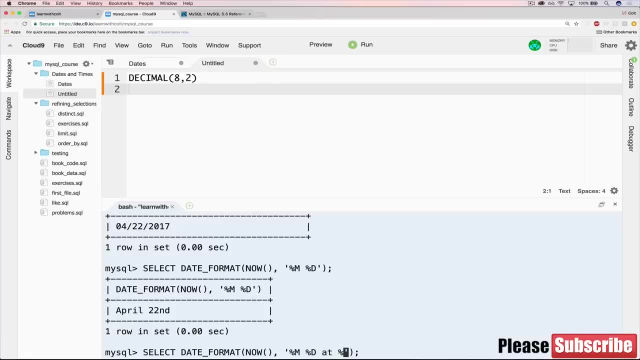 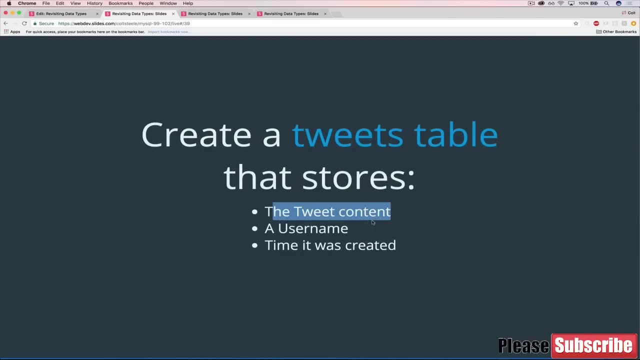 Okay, So lowercase h, colon, lowercase i: There we go. April 22nd at 4.15.. Great. Now, moving on to our final problem: Create a tweets table that stores the tweet content, a username and the time it was created. 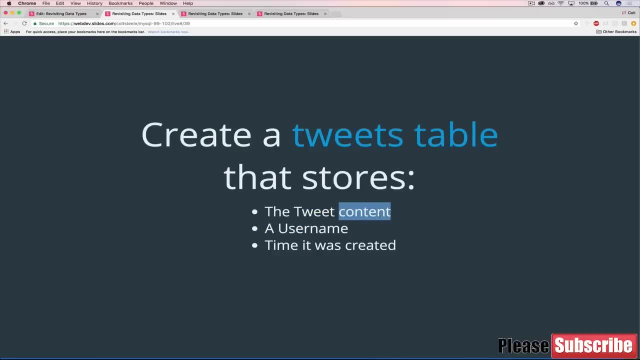 So the tweet itself can vary in length, so it should be a varchar most likely. A username could vary in length as well, And then the time it's created could be a date time. I mean, it could just be a time if you wanted it to. but what makes the most sense? 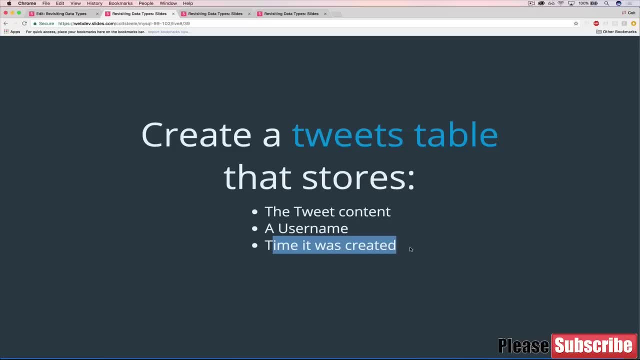 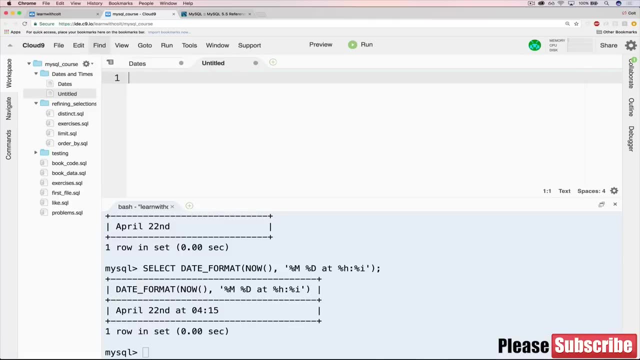 we discussed already is to use timestamp, And we want to set the default to be now. So let's try it. Let's hop over here and the first thing we want is a create table tweets, and then we're going to have 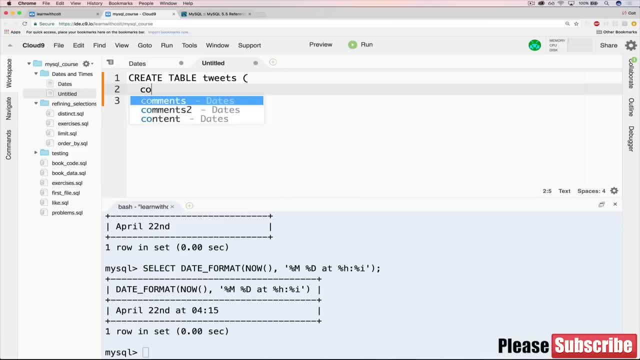 tweet content. so we could call that whatever we want, I'll just call it content. That will be a varchar up to 140 characters. Then we have username, which will also be a varchar up to 20 characters, And then, finally, we have 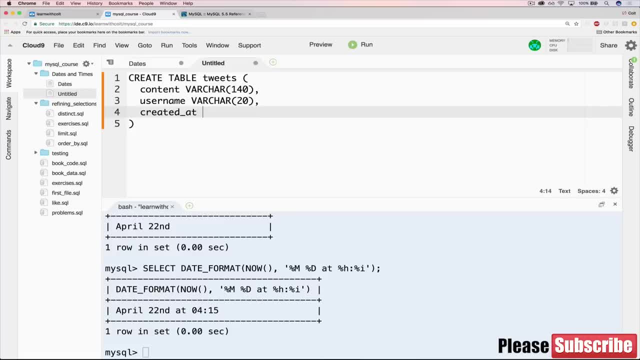 created at or tweeted at, or time, or whatever you want to call it, which will be a timestamp. And then the important part is default now Or default current timestamp, but I like to use now, So let's try it. 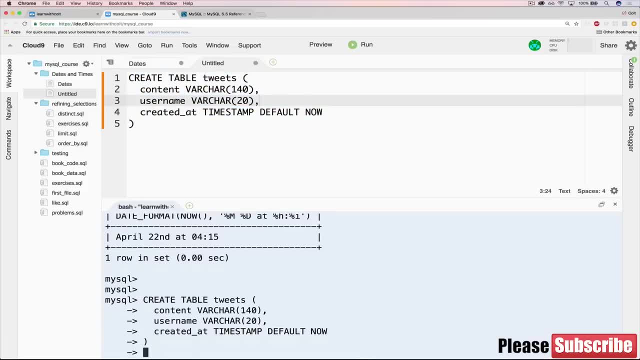 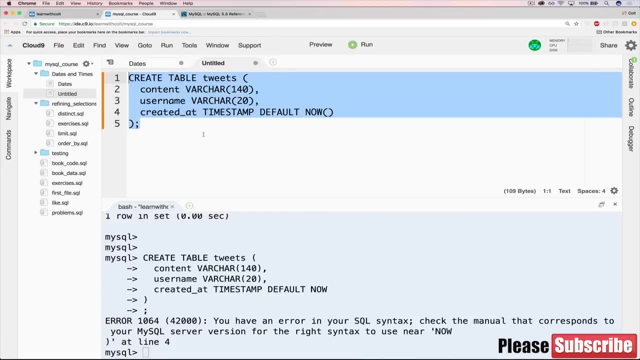 see if it works. Make sure we have the right commas in place: Semicolon- And good thing we tried it. Parentheses around now. Add the semicolon in as well. Okay, make some space. Now we run it. 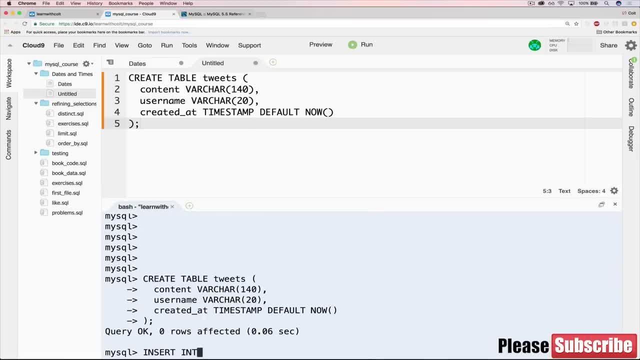 and it appears to work. Let's just make sure by inserting one tweet, So we'll do content. username, remember, we don't need to insert. created at manually And let's see. content will be. this is my first tweet And username will be. 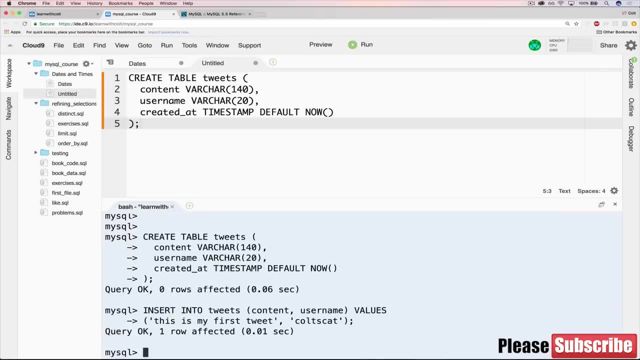 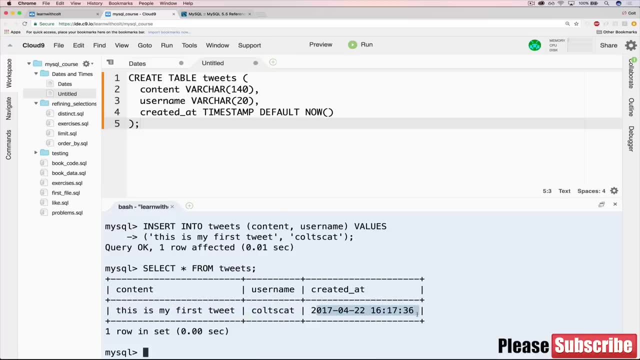 coltscat. Okay, let's do a select star from tweets And you can see. we have created that in there as a timestamp. Works perfectly. Just double check by inserting something else. Let's just change it slightly. This is my. 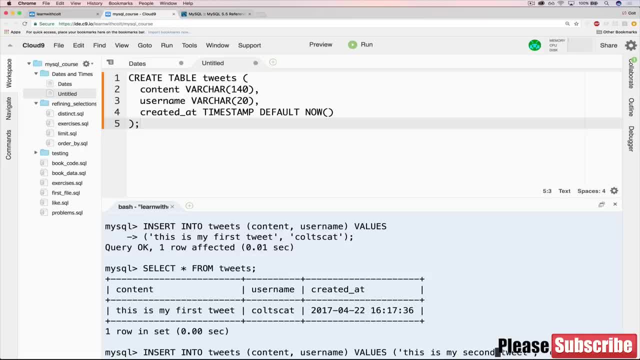 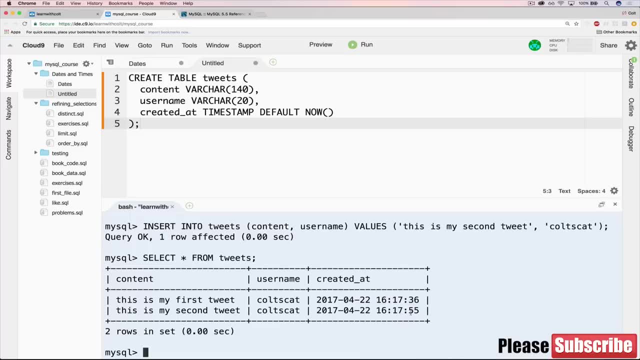 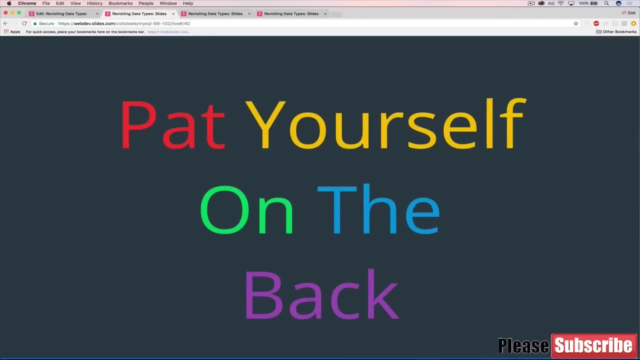 second tweet. Now, if we select star, two different timestamps, Just a couple seconds later. Okay, now the hardest part: Pat yourself on the back. You made it through. Siri, can you say hello? Hello, it's me. I was wondering if. 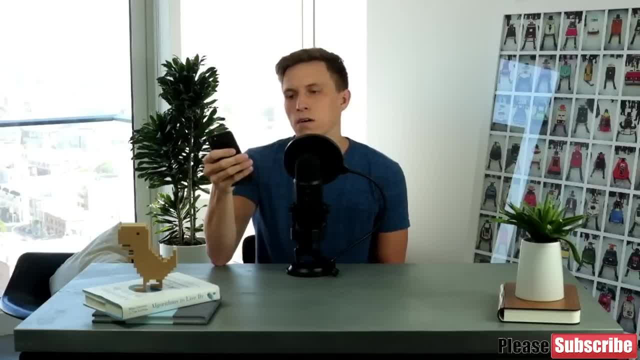 after all these years, you'd like to meet To go over everything. They say that time's supposed to heal you, but I ain't done much healing. Okay, thank you, Siri. Can you just say hello, not sing it? Hi Colt wants me to say hello. 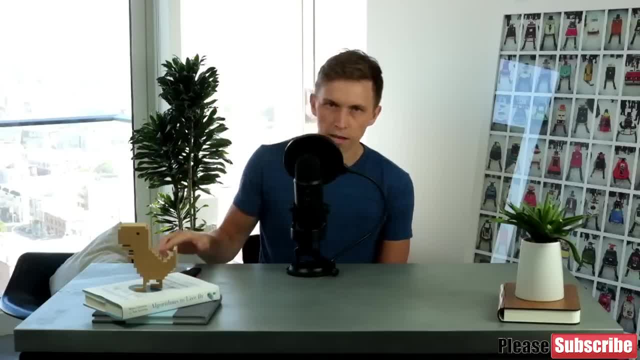 and welcome to the next section. Thank you, Siri. So, as Siri said, hi, welcome to the next section. This section is all about logical operators, So if you come from a programming language or have any programming experience, you have probably stumbled across. 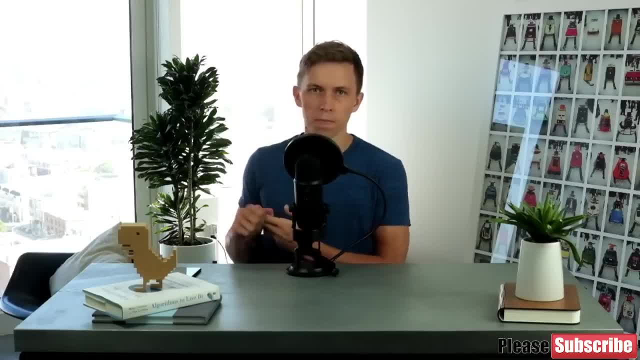 logical operators, Things like logical AND and logical OR. There's a bunch of others, but those are the primary two. If you haven't, if you have no idea what I'm talking about, don't panic. That's what this section is all about. 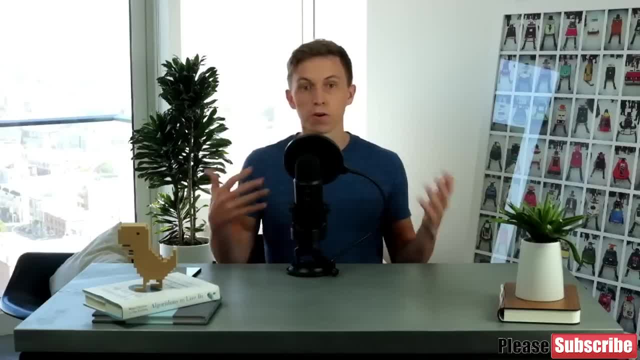 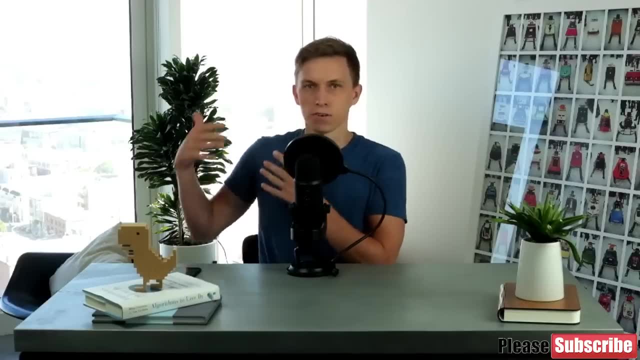 So this will either serve as a review if you know how to program or if you know logical operators, and it will serve as a way to show you how they work in MySQL, or it will serve to both introduce them and to show you how they. 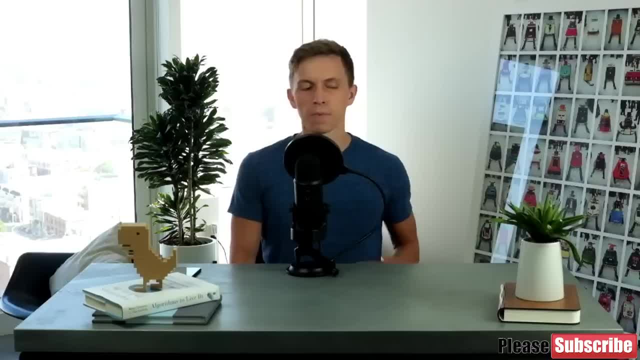 work in MySQL. Either way, they're really powerful. I'm not going to say they're important. they are important, but I'm just overusing that phrase. in these videos. Everything's important here, But these allow us to string together different. 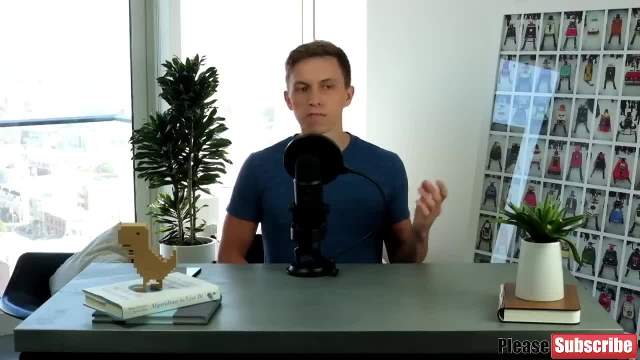 queries and make more complex selections. So if I were to give you a really contrived, idiotic example like cars and I want to select all cars based off of a color, Right now all we could do is select all cars that have a color of. 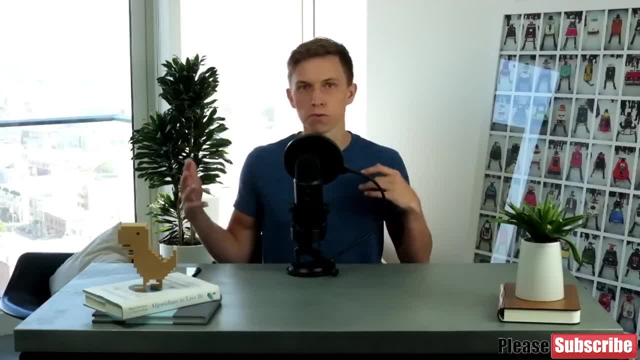 exactly blue, or a color that contains the word blue, like I don't know, sky blue or seashore blue or something like that. That's fine, but what if you also wanted to select all cars that were blue or that were red? 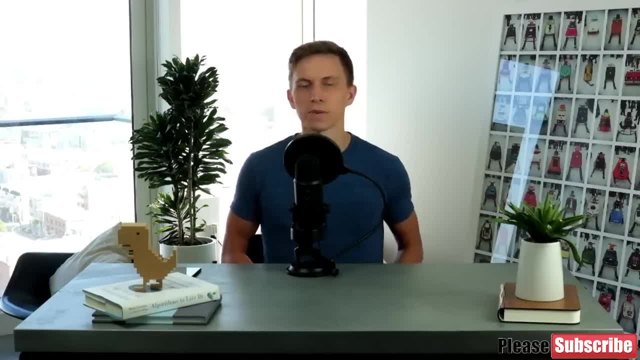 Again, I said contrived and silly, but the idea is we can string things together. So, rather than having to do two queries, we could put them together, Or if we go to our books- example which, by the way, we're about to finish with, this is the last of that. 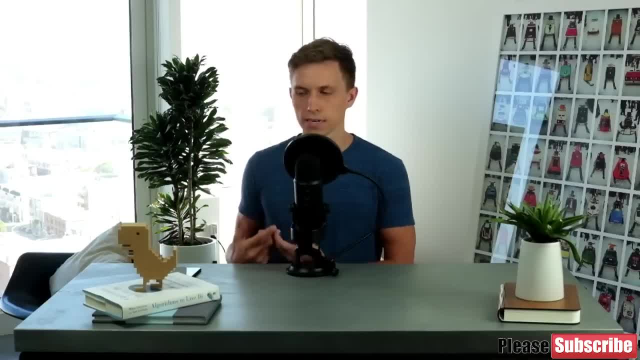 section last of our books data. we could make more complex selections, like select all books that have a price below $20 and at the same time, they're I don't know. we have 50 copies in stock. Or we could do something like select all books. 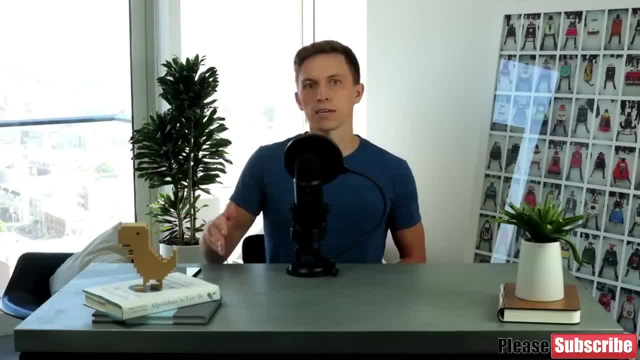 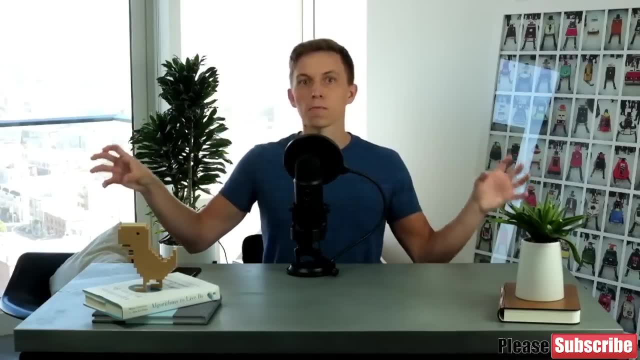 written by a certain author before the year 1990.. So two different components. right, We could select all books before 1990, select all books written by a certain author, but put them together. we need to use a logical operator. 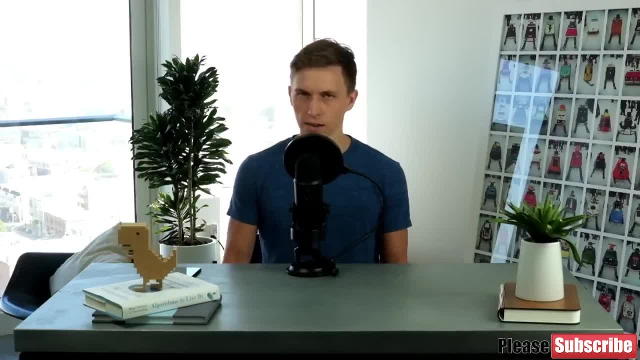 Alright, I'm rambling a little bit, I apologize. This section is on logical operators. Lots of exercises, of course, like always. Hopefully they're enjoyable. If not, well, like I said, it is a course on databases, so 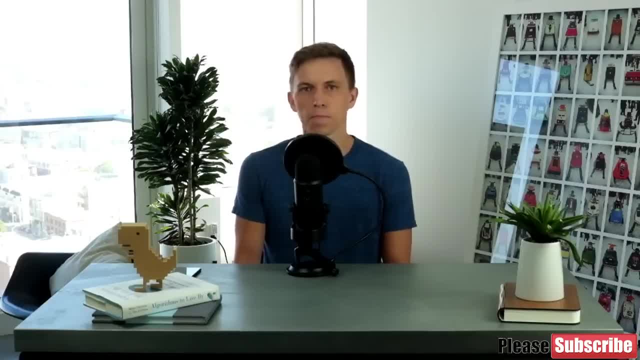 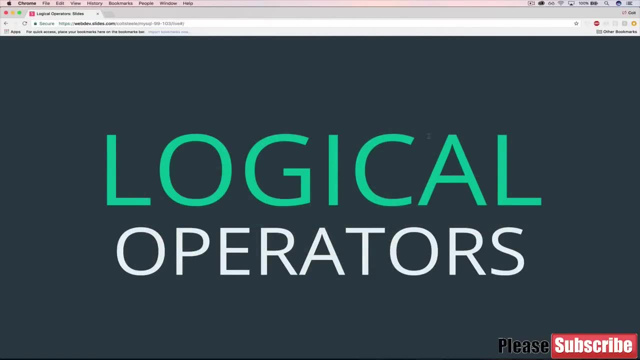 I'm trying, I really am. Yeah, Okay, I'm gonna stop. So in this section we're gonna focus on what are called logical operators. Actually, we're focusing on operators in general, and most of the ones we're gonna work with are logical operators. 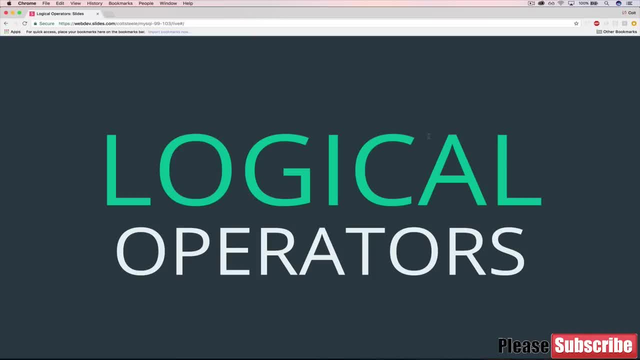 That distinction doesn't really matter, though. I'm just gonna call them all logical operators, And they allow us to add logic into our SQL statements. So up until this point, we've seen things like well, like-like, which allows us. 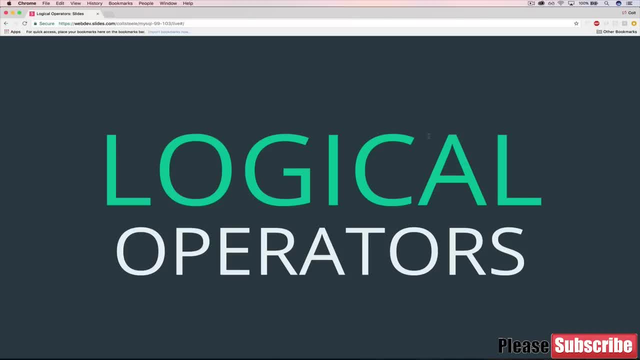 to select things based off of text, looking or containing certain strings, matching patterns. We've seen how to do things where we can check, you know, select all books where the title is exactly, uh, Lincoln and the Bardo, or where release year is. 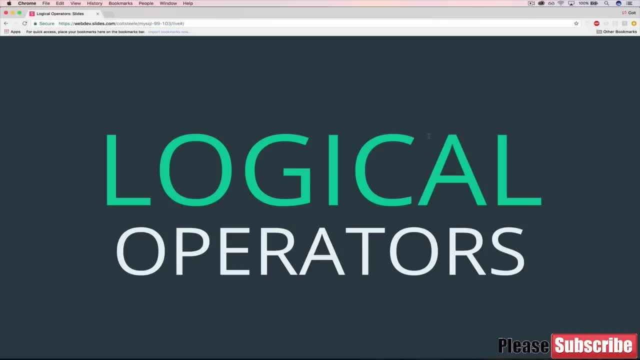 exactly 2013.. But there's a whole slew of other things that we'd like to be able to select based off of um, and that's what we're gonna focus on in this section. So we're gonna see how to do things like 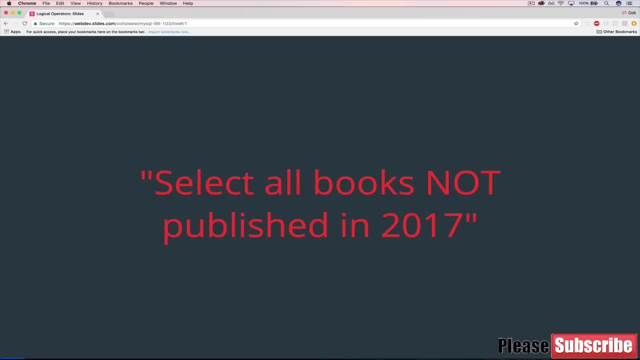 select all books not published in 2017.. Right now, we don't have a way of doing that. Or what about select all birthdays between two different dates, So not just all birthdays that are exactly, you know, April 22,. 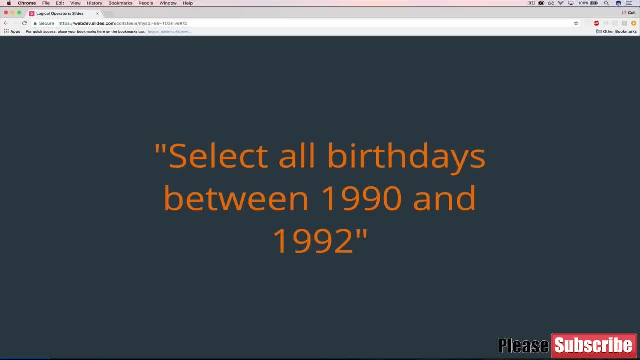 1990 or 1992 or whatever it is, but between those two dates Or select all items. so this is some table I made up called items all items that are in stock and priced below $19.99.. So that's two different things. 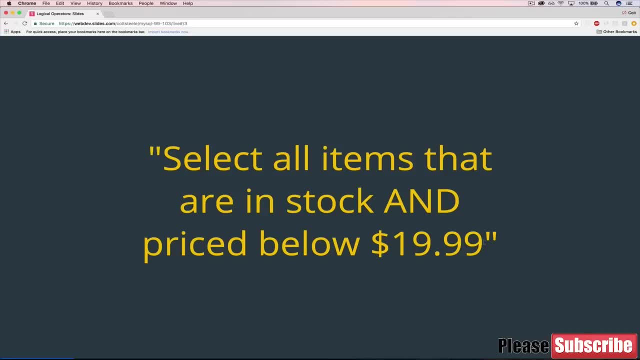 We know how to select all items that are in stock, but there's a second component, which is: not only do they need to be in stock, but they need to be priced below $19.99. And right now, we don't know how to do that either. 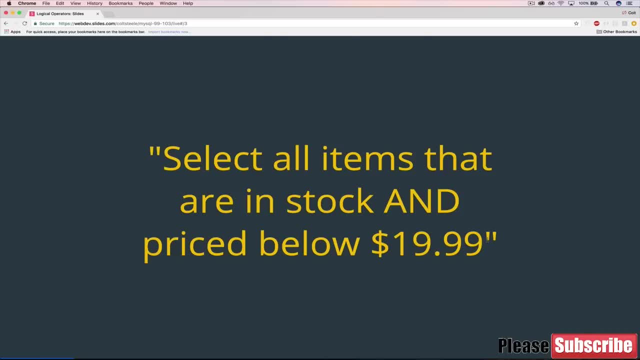 With that lengthy introduction out of the way, let's take a look at some of our first ones. So the actual first one we're gonna look at is called not equal, And it looks like this Exclamation point and an equals sign. So we've seen how to do things using. 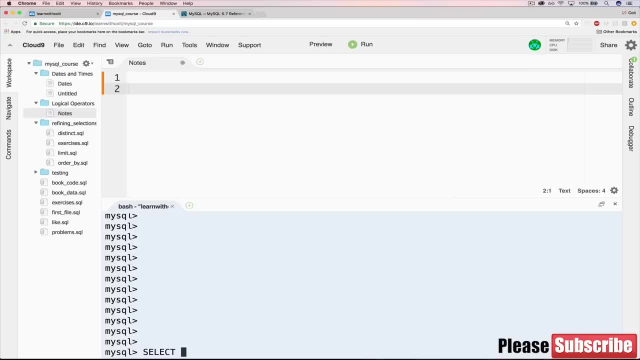 equals sign right, We've done, you know, select, let's do title comma, released year from books where, and let's do released year so where released year is exactly 2017.. So we've seen how to do this, you know. 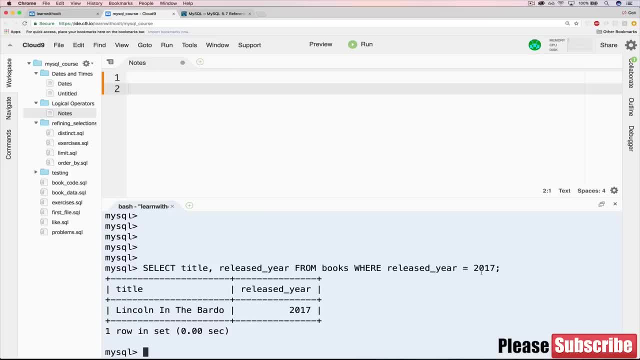 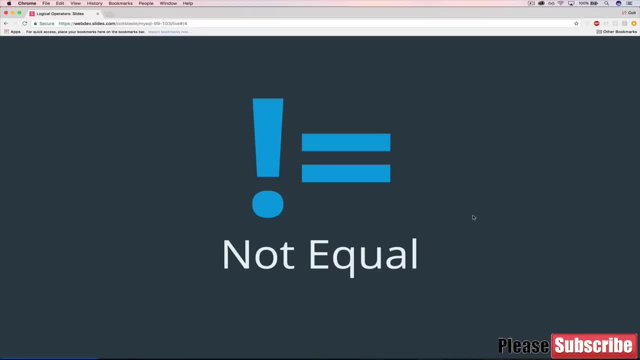 with the equals sign. We've been doing it all the time. However, what if I want to do the opposite? I want all books that were released in any year excluding 2017.. So what we want to do is basically replace that equals sign. 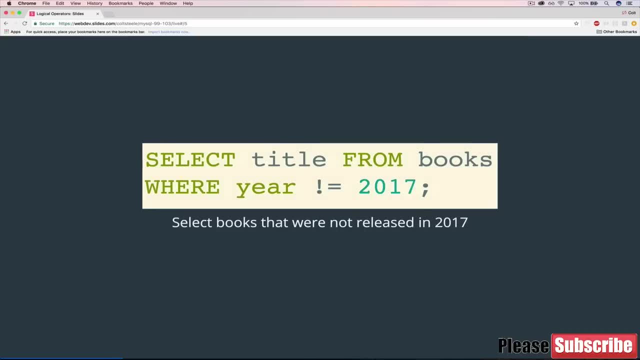 with a not equals. So we could do this: Select title from books where year is not equal to 2017.. If you're familiar with any programming languages, you've probably come across this not equals. It's a pretty universal way of writing not equals, So let's give it. 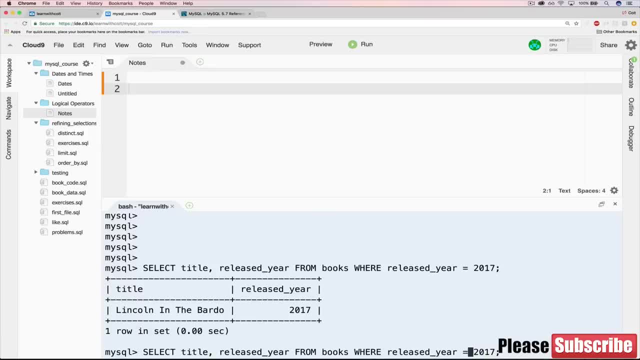 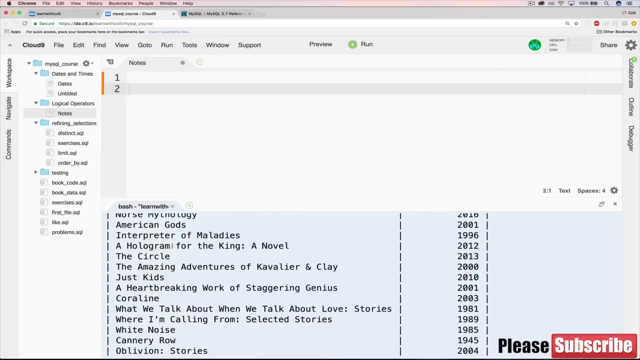 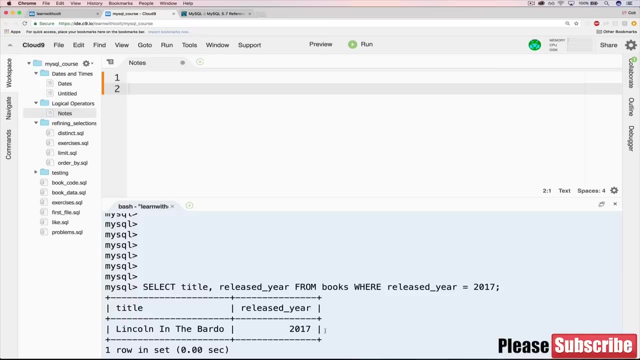 a shot. Recall this and just replace it with not equals, And now you can hopefully see that we get everything back except for Lincoln and the Bardo. And, of course, if there was more than one book released in 2017, then we would get any book back or all books. 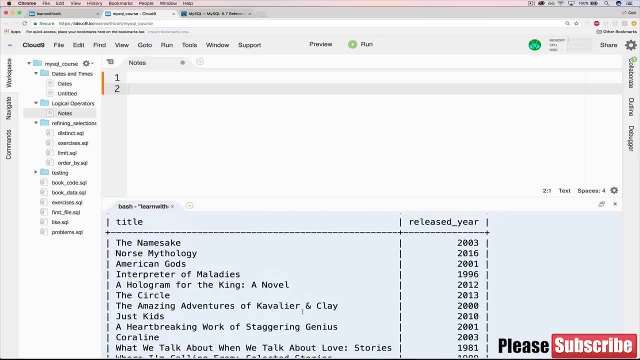 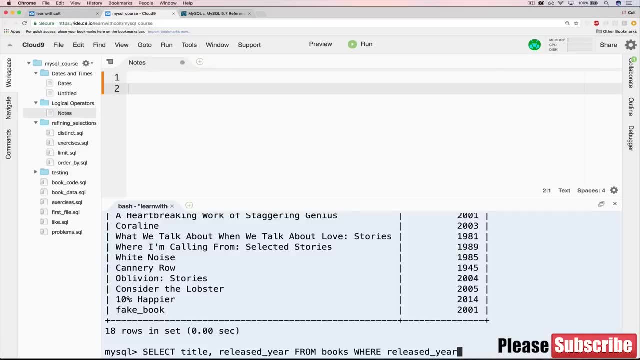 back, except that those books from 2017.. So we can see that it's gone. We could do the same thing, but instead of working with released year, what if we do it with author? So let me just start over here. Let's select. 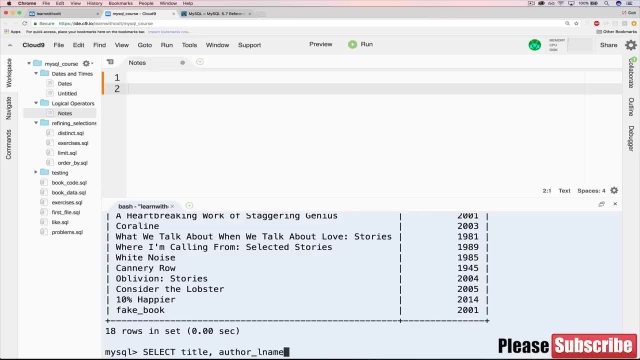 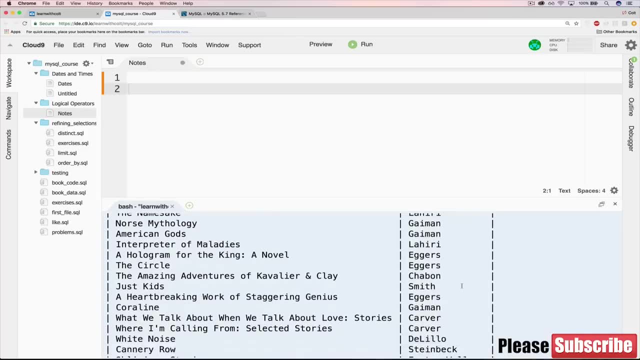 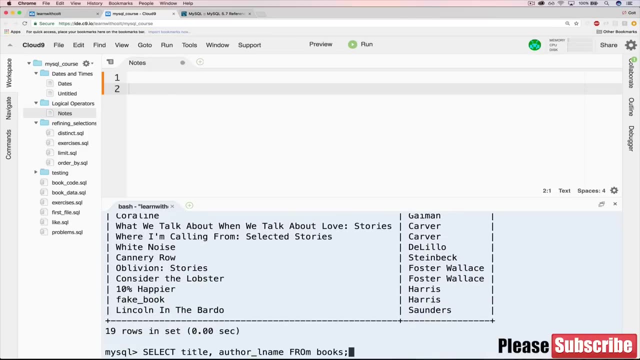 title and author last name from books, And we'll start just with all of them, And then let's select where author last name is exactly equal to Harris. So we have those two Harris's Where author L name equals Harris, Just like that. 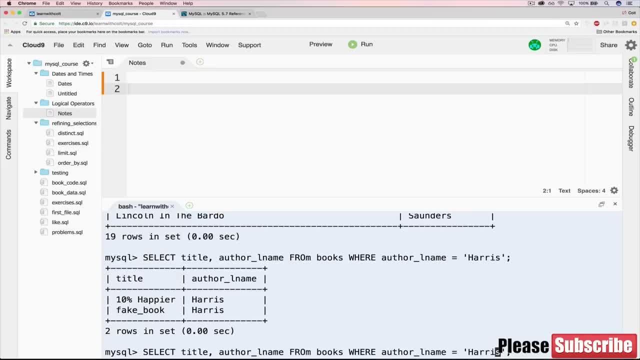 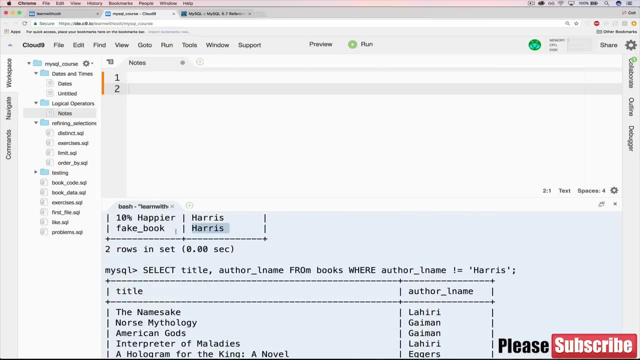 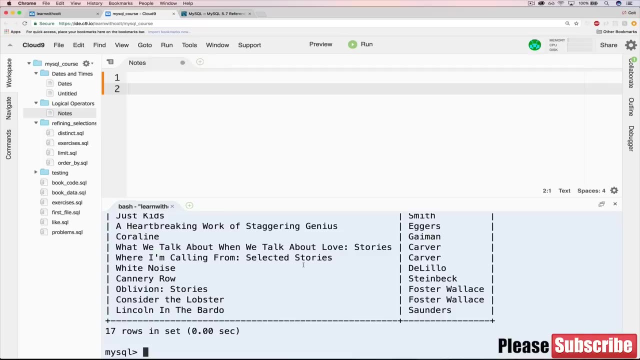 And we get those two, And by just flipping the switch here, that exclamation point, we now get everything except those two. Okay, So hopefully you get the point by now. Equals works like you would expect If you're not familiar with the exclamation point. 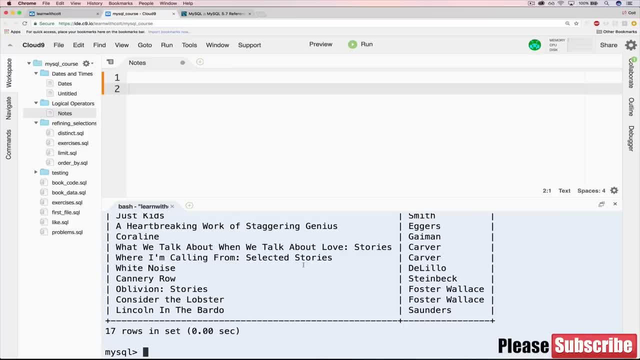 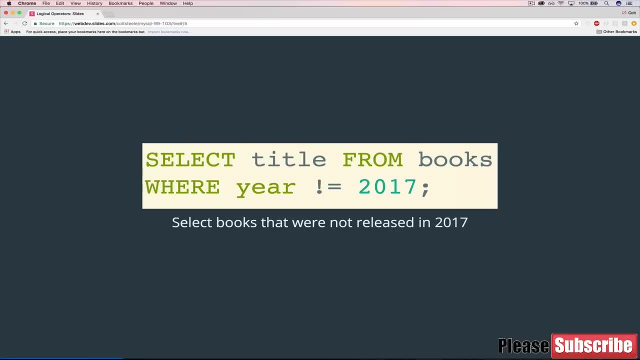 it might take a little bit of getting used to, But otherwise it's pretty straightforward. It's the opposite of equals Awesome. So that's the first one that we're taking a look at, but we have quite a few more. Next up, we're going to talk about something. 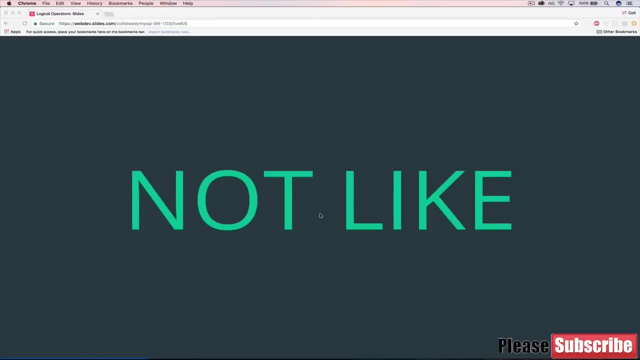 very similar, which is not like. Okay, So we saw not equals, which is the opposite of the equals sign. Now we're going to look at not like And, as you probably guessed, not like is the opposite of like. So, just to review, we haven't used 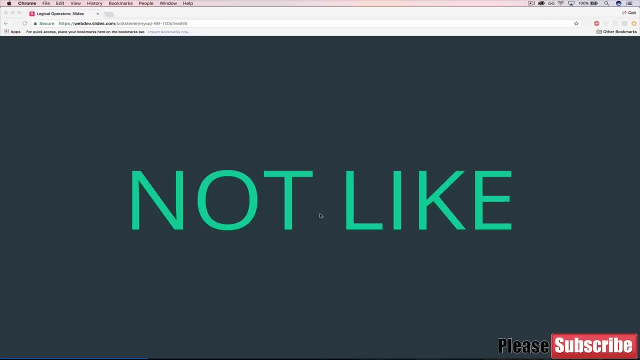 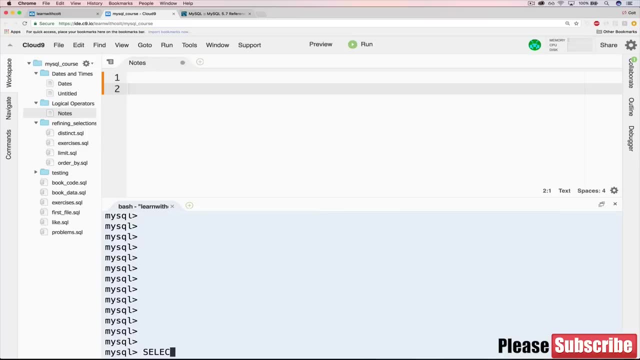 like all that much, but it is a pretty common and important one. It allows us to match patterns in strings usually, So we can do things like select- let's do all titles and we'll just do title from books where title like. and we can do things like: 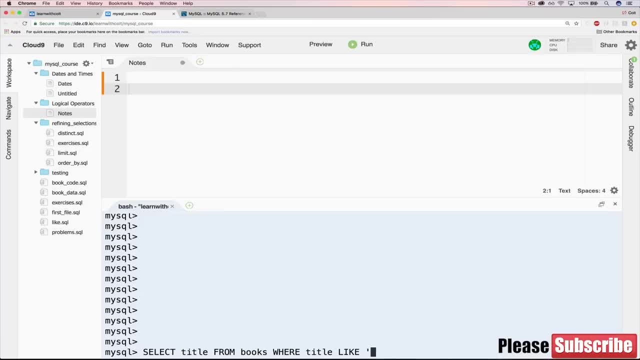 we'll start off. how about all books that contain, how about all books that start with the letter W, Just like that? And if we just do W on its own, remember that doesn't really give us anything, unless it's an exact match of the letter W. but 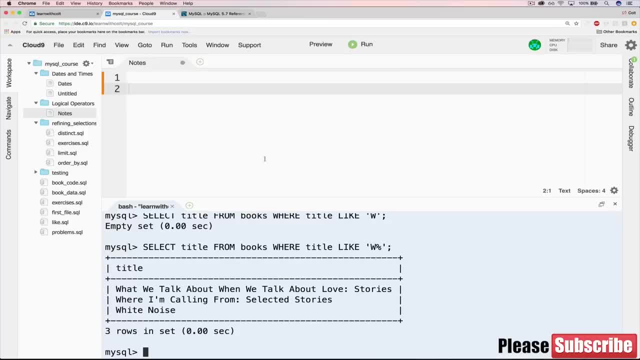 we use the percent sign there as a placeholder, And now this says all books that start with the letter W and anything afterwards, or we could expand that to be any title that has the letter W. Okay, So that's it for review. That's how like works, We match. 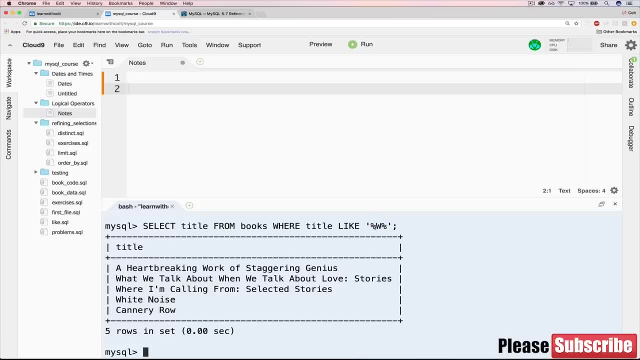 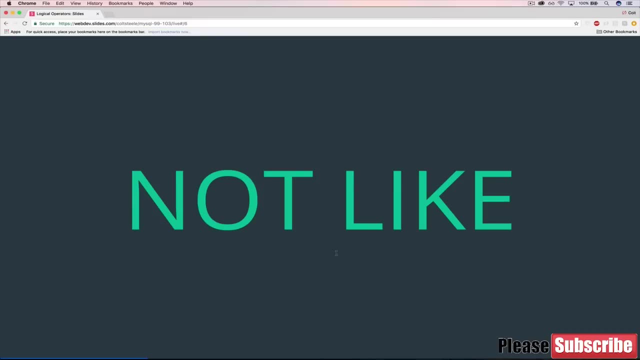 these patterns and anything that matches this pattern, where these are placeholders, the percent signs, I mean. anything goes there, Anything that matches this, will be returned. So all of these contain a W somewhere. Alright, So that brings us to not like, which, as you have probably, 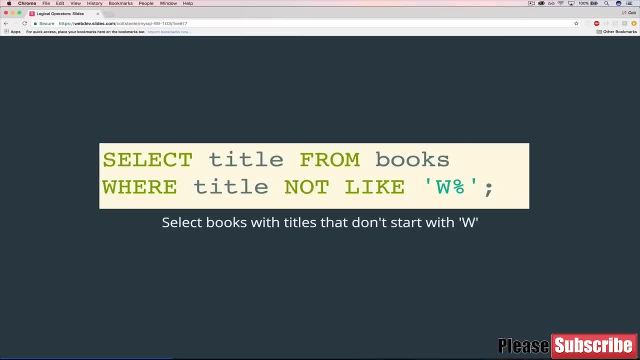 surmised by now, it will do the opposite. So here's an example: Select all books with titles that don't start with the letter W. So rather than the exclamation point equals, like we had for not equals, we just use the word, not space. 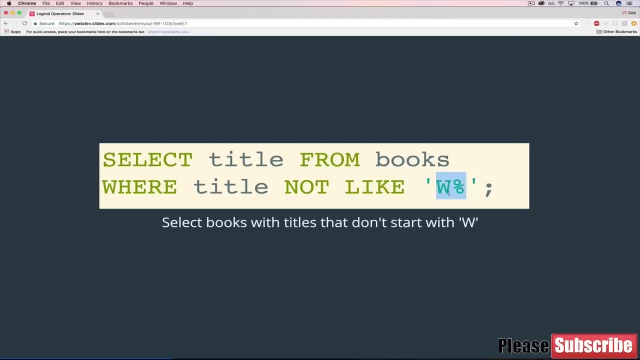 like, And then in this case, W percent sign means something that has a W and then anything after that, And then we're negating that with not. So this in effect says: select all the book titles that don't start with the letter W. So if we go back, 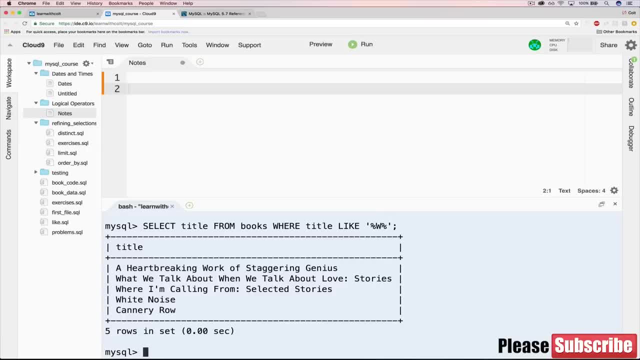 recall this, which gives us these. well, actually, let me get rid of the percent sign at the beginning. These are the three books that start with the W. What we talk about when we talk about love. where I'm calling from, and white noise. 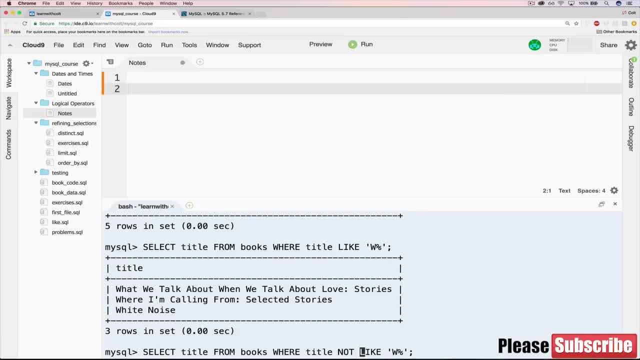 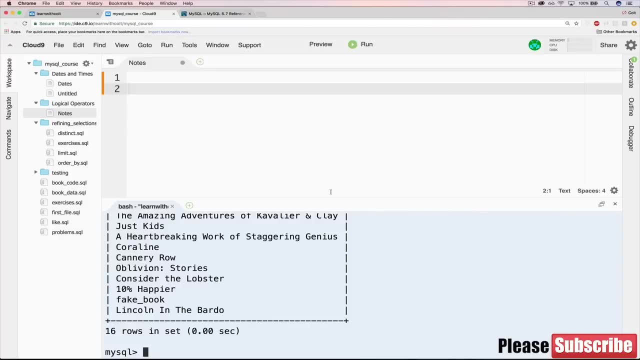 And if we go and just add- not now- we get all book titles excluding these three. Alright, so that's it for not like. Hopefully you liked that rather than not liked it, I guess. Alright, well, let's just move on. So next up, we're moving. 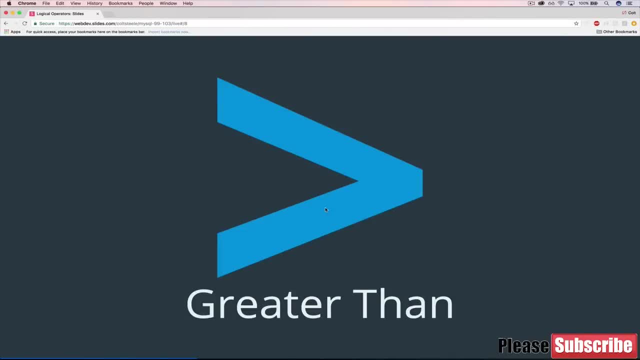 on to the next subset of logical operators. There's a group that fits together now, Which you're probably familiar with just from middle school or early school years, And those are the greater than, greater than and equal to, or sorry, greater than or equal to less than. 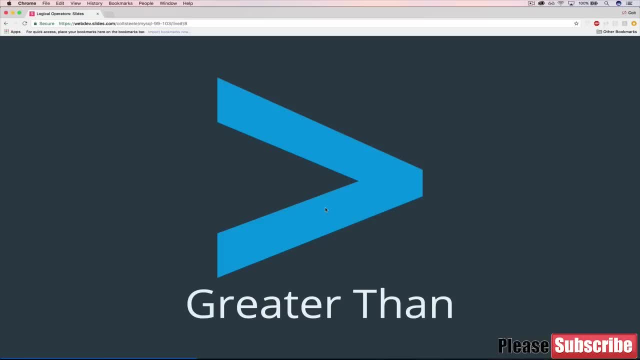 and less than or equal to. So four operators very similar and pretty useful. So this is the greater than operator in MySQL. It's pretty standard. The. what is this called? the alligator bracket? I don't know what to call this, honestly. I just call it the. 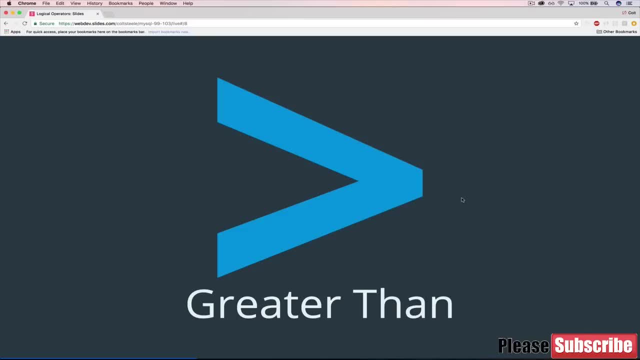 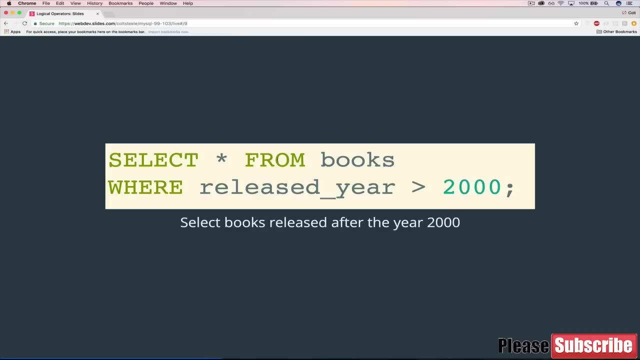 greater than bracket. It's pretty universal across programming and it allows us to do things like select all the books released after a certain year. So select all books where released year is greater than the year 2000.. And typically we're working with numbers I'll talk about 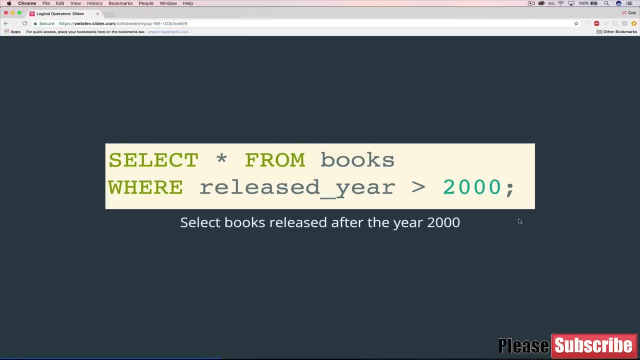 strings in a little bit, but typically we're working with numbers. So an example: earlier today I was looking on Airbnb to book an Airbnb and they have a filter that allows you to set a minimum price or a maximum price. So if I wanted to, I could have gone in and said I only 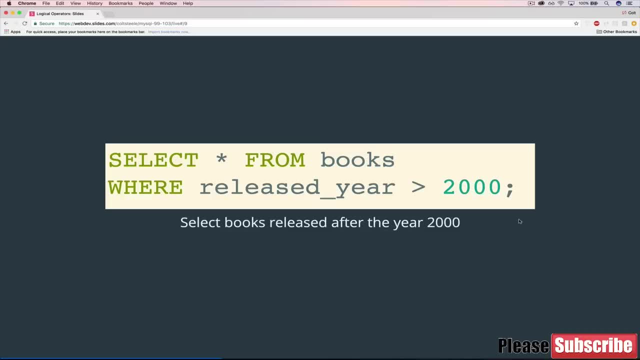 want to book. you know Airbnbs that have a price greater than $50 a night or something To filter out the $20 a night. you know couches in some person's living room, So that's powered behind the scenes, most likely by. 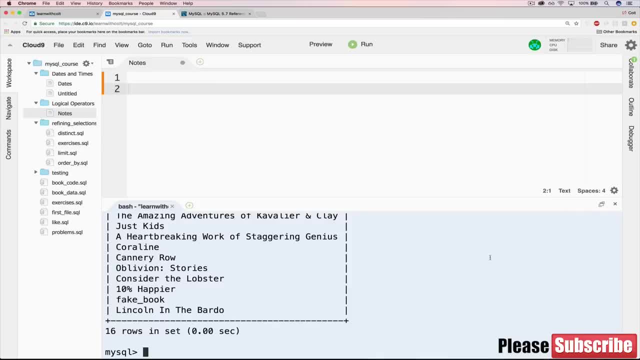 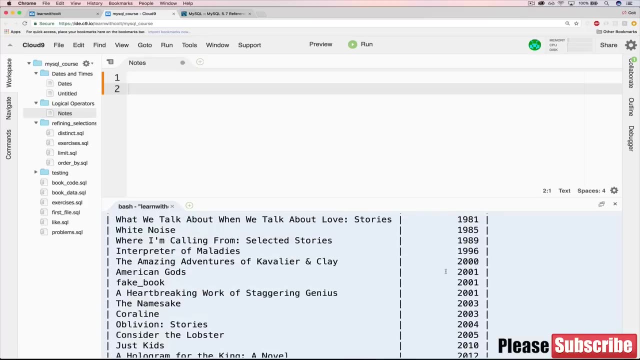 a greater than sign. So now let's give it a shot on our own. If we hop over here, Let's start by just selecting all titles and released year from books and let's just order by released year. Just ordering it will. let us see. 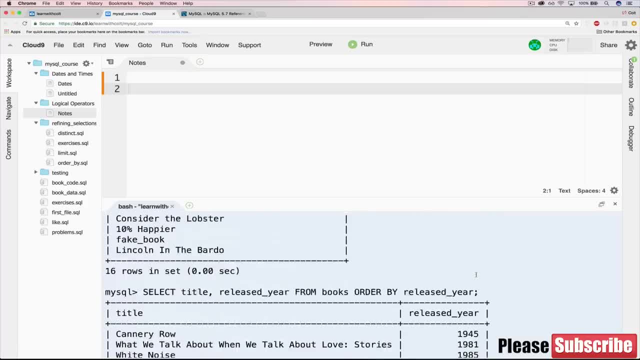 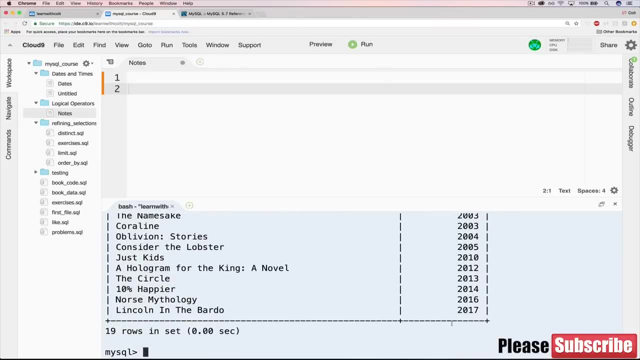 you know, when we remove things, It will make it clearer rather than having them just be jumbled. Okay, so we've got 1945 up to 2017.. Now, if I want to go ahead and do what I showed you, which is select all the books, 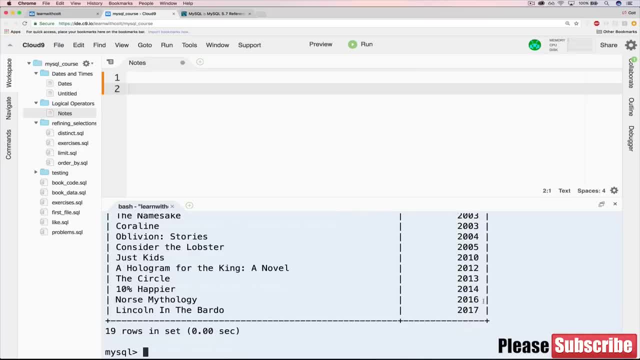 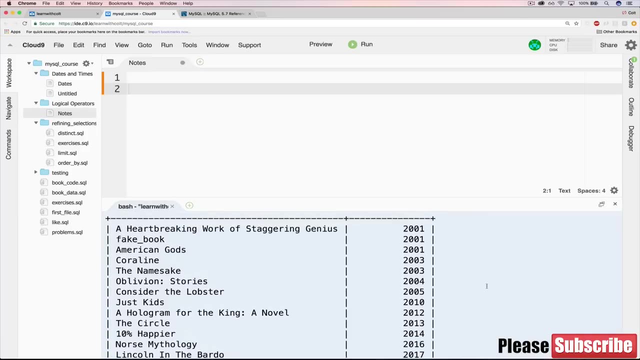 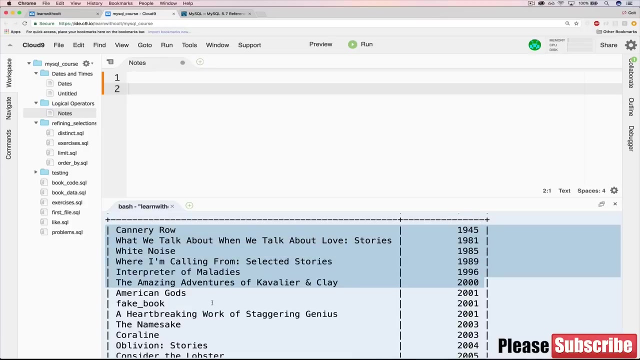 released in the 2000s or after the year 2000. all I need to do is add in where released year is greater than 2000.. Just like that. And if we look, we lost everything from here on back. So from Cannery Row to The Amazing Adventures of Cavalier and Clay. 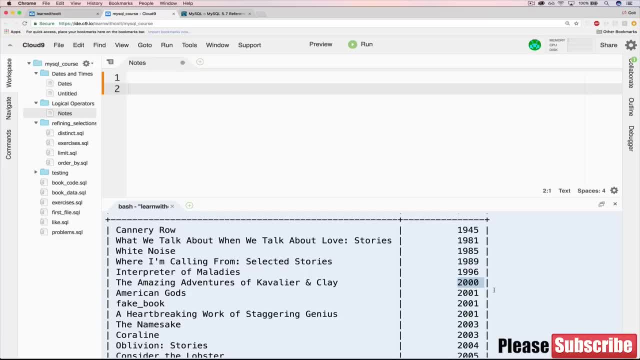 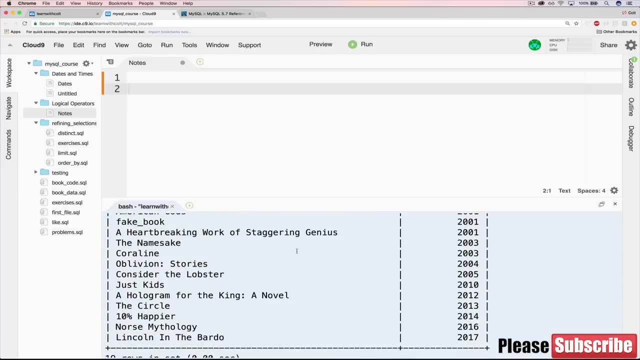 Important to note that 2000 is not included, which we'll get to in just a moment, But everything greater than 2000 is. So that gives us all of these books, from American Gods down to Lincoln and the Bardo, As you can see. 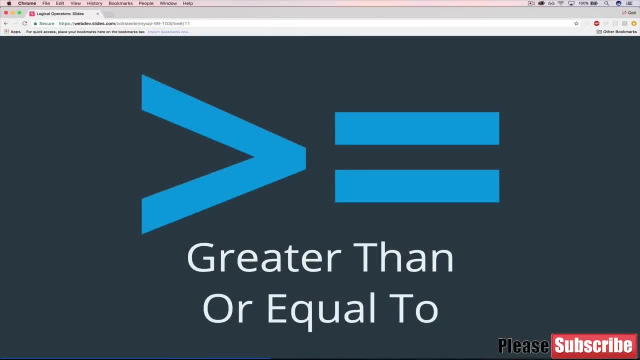 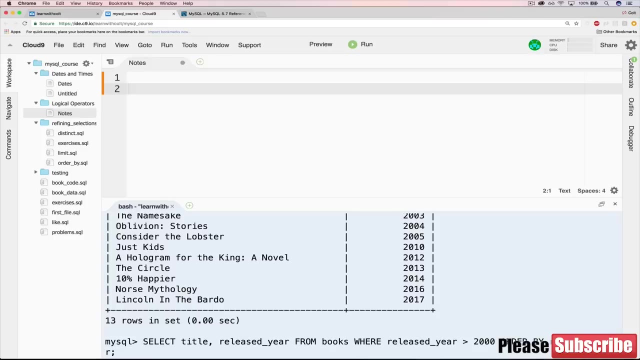 Here we go. So that brings us to greater than or equal to, which works exactly the same way, except you add in this equal sign afterwards, which makes it rather than greater than. it makes it greater than or equal to, which means that it's inclusive. So if I just change that, 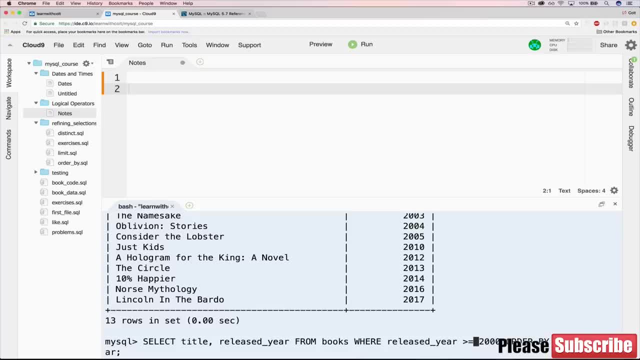 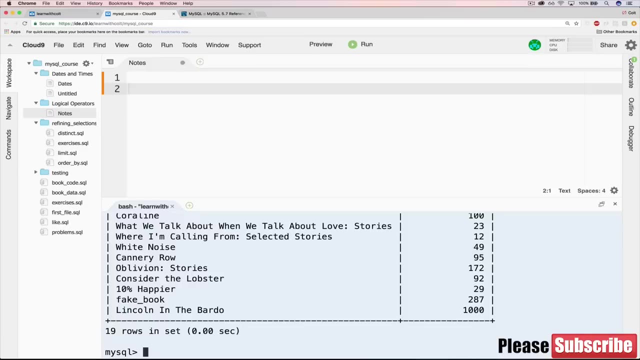 and do where released year, rather than greater than, is greater than or equal to 2000. now it includes the year 2000.. Let's do one more quick example. Let's do a select title and stock quantity from books And let's say that we're going to do a sale. 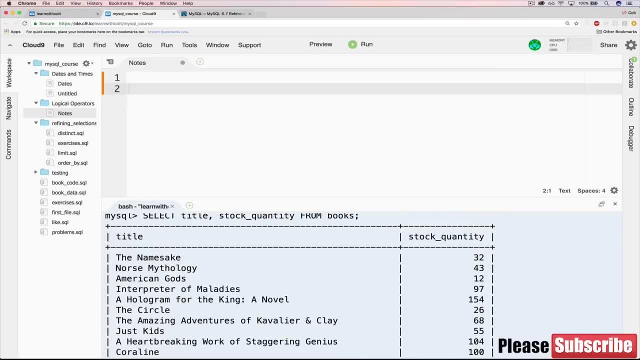 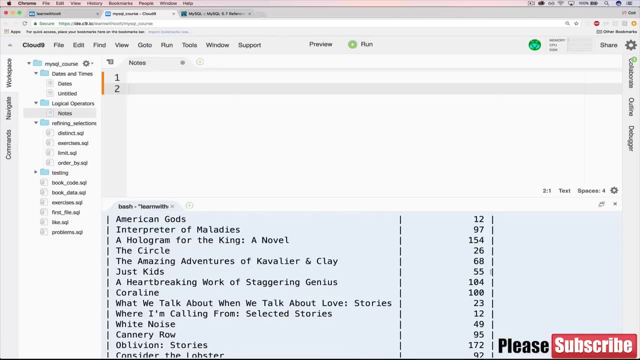 because we have some excess stock in some of our books, Any book that we have more than 100, including 100, let's say So 100 or more copies in stock. we want to select and we're going to discount them. So how do we select those? 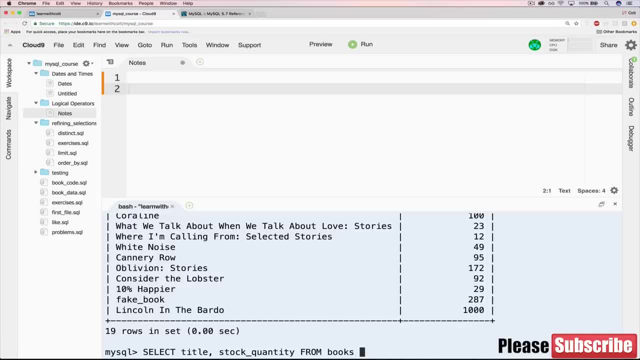 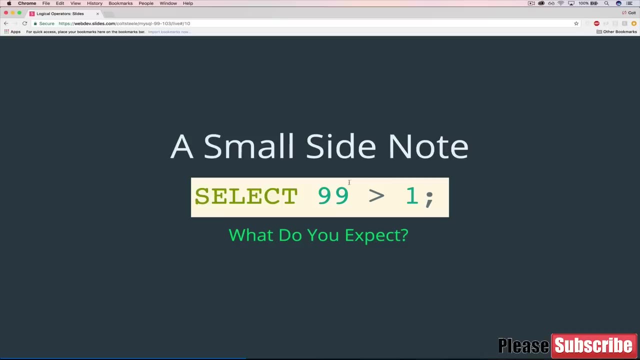 Well, it's pretty straight forward. We're just going to select title and stock quantity from books where stock quantity is greater than or equal to 100.. And there we go. These are the books that we're going to discount. Alright, Okay, so there's. 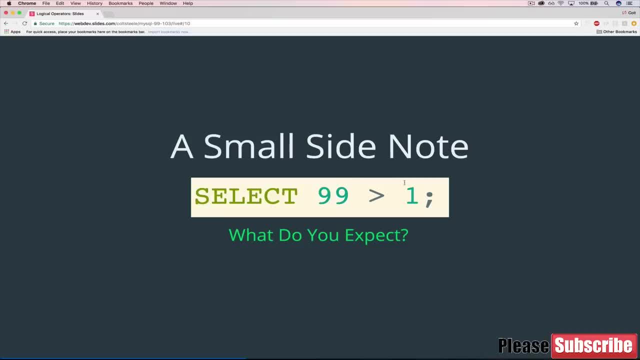 one other small tangent I want to talk about. It's a bit of a diversion away from the tables and books that we've been working with. This has nothing to do with any particular data, But if you try running something like this: Select 99 greater than 1.. 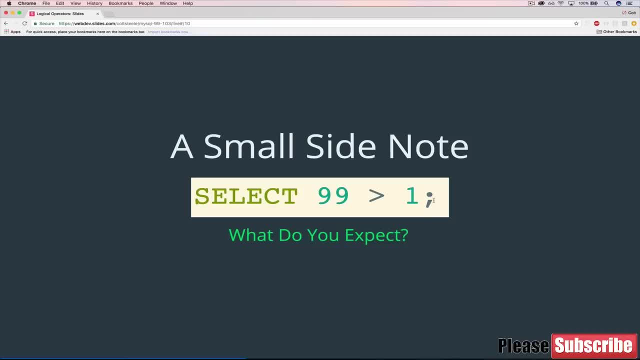 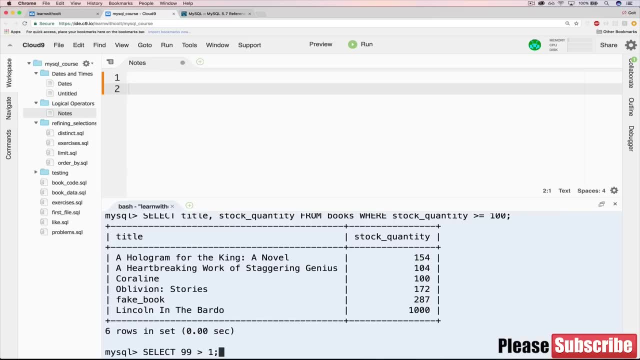 What do you expect? Well, go ahead and try it. if you'd like, I'll go and type it over here. Select 99 greater than 1.. If we hit enter, we get the number 1 back. Alright, so if you're familiar with, 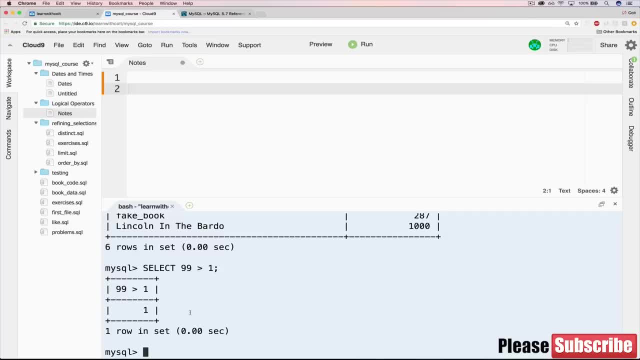 other programming languages, you've probably come across Boolean values- True or false values- And that's what MySQL is replicating here. So the way that it works in Boolean logic is it actually works with the numbers 0 and 1.. So we know that. 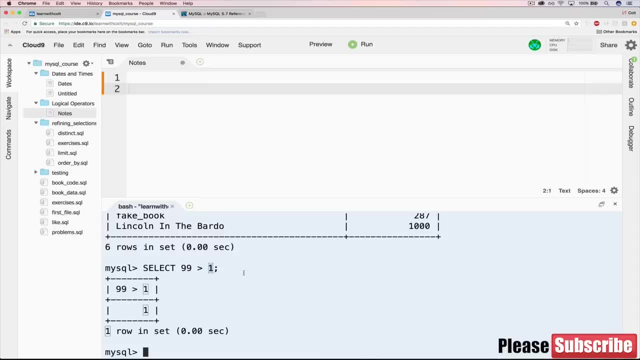 99 is greater than 1.. That's true. So we get 1, which is equivalent to true. Basically, this evaluates to 1, which you can think of as evaluating to true. So if that's confusing you, let's try something. Let's change 99. 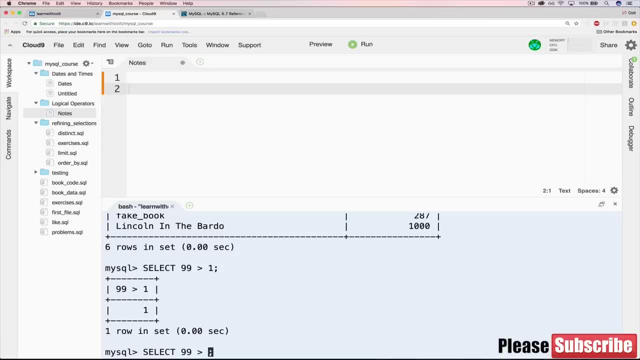 greater than 1 to is 99, greater than 567.. I just lost it. Here we go. We know that that's false And you can see we get 0.. So the reason that I'm showing this to you, well, there's two reasons. 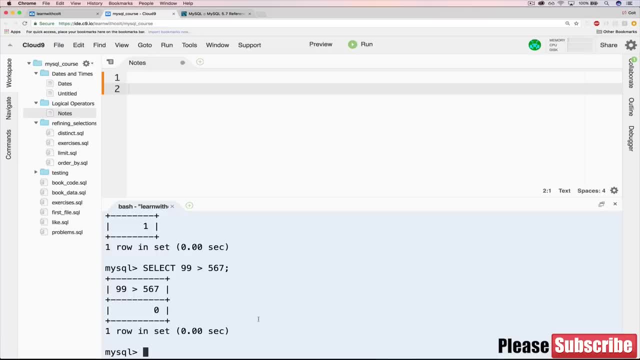 One is that it will help us going forward with some of the other things I'm going to show you. When we can start chaining things together, you'll be able to evaluate them and kind of do some exercises on your own first. But the other thing- 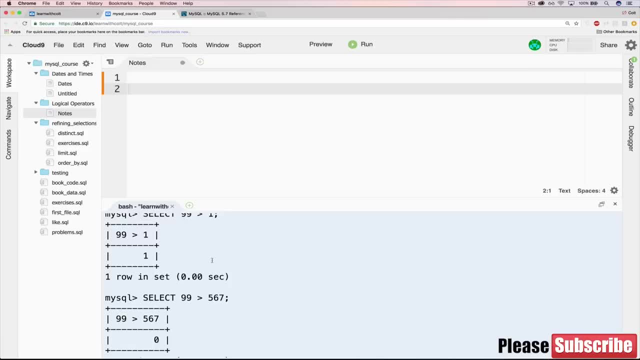 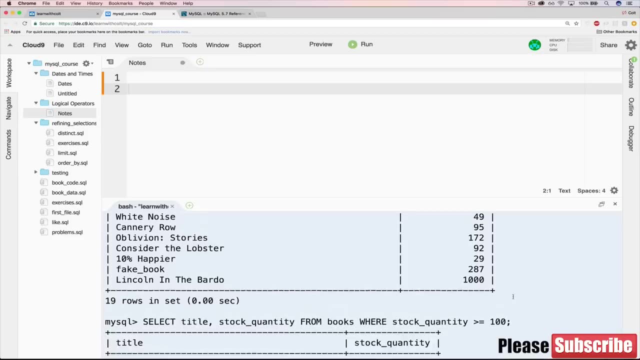 and the more important reason is that this is what's happening behind the scenes. When we have something like this right here, Where stock quantity is greater than or equal to 100, you can almost think of it as MySQL going through every stock quantity and plugging it in here. 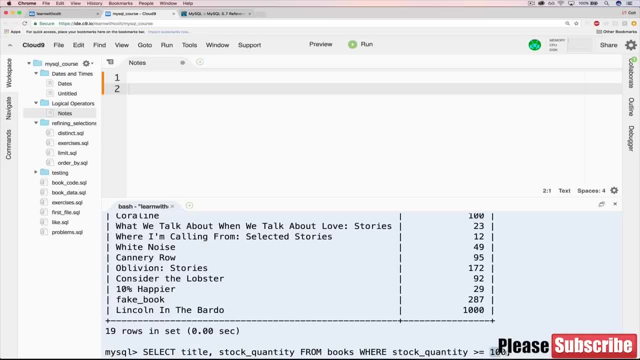 and trying: Okay. is 100 greater than or equal to 100? 1. Yes, Okay, So keep that one. Is 23 greater than or equal to 100? 0. No- False, So get rid of that one And it does. 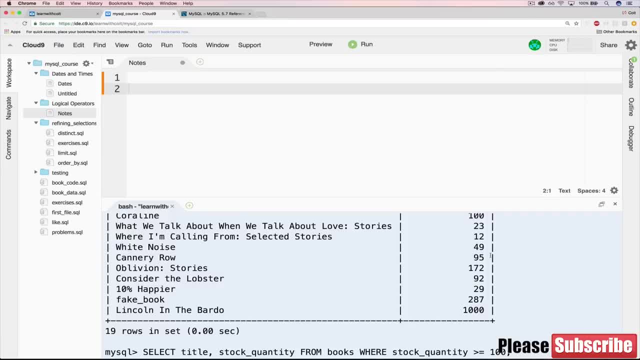 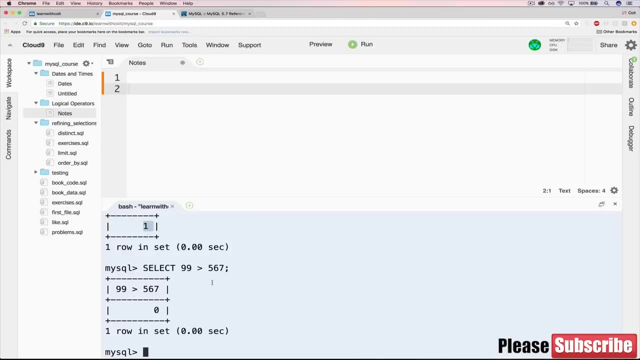 that going down the line. That's kind of the humanized version, if you will, But it's evaluating to these numbers, But those numbers are just bits in memory, But the concept is this. It's the same. So, if you'd like, let's wrap this up with. 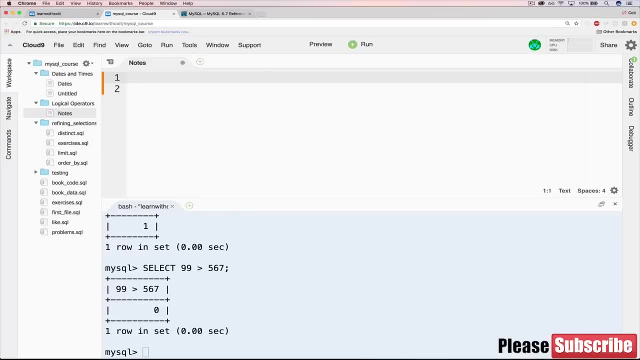 just a really simple exercise. I'm going to type up a few things and I'd like for you to evaluate them yourselves. Okay, So I typed up a couple of examples here And I'd like for you to just either mentally try these or actually try them yourselves. 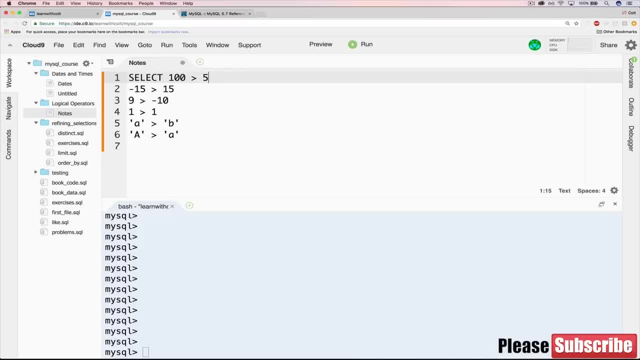 And remember, you'll need to actually run select and you'll need a semicolon. But what's the result that you expect? And there are a couple of straightforward ones, And then I just threw in two string ones at the end, basically to give myself a talking. 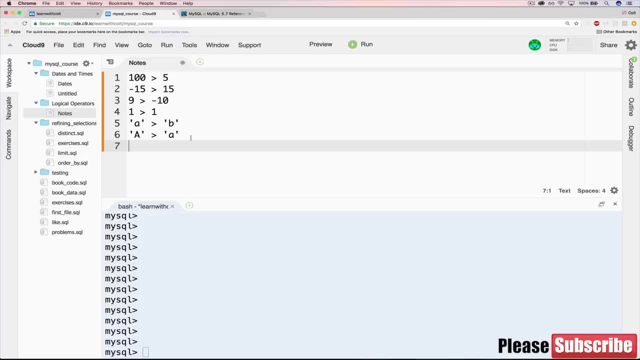 point at the end, I want to talk about why this happens and, if you should care, So go ahead- I'll throw up a thing on the screen that says you should do it, And then in like two seconds I'll be back. Alright, I'm back. 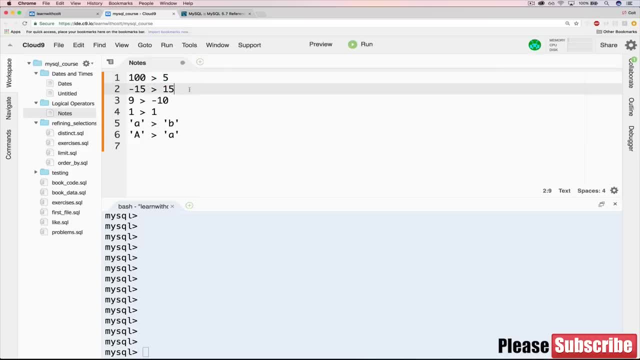 So, first one: 100 greater than 5.. Is that true? Well, yes, I believe that to be true. Just to double check, It gives us 1.. That means we're in the clear Negative: 15 greater than 15.. Is that true? 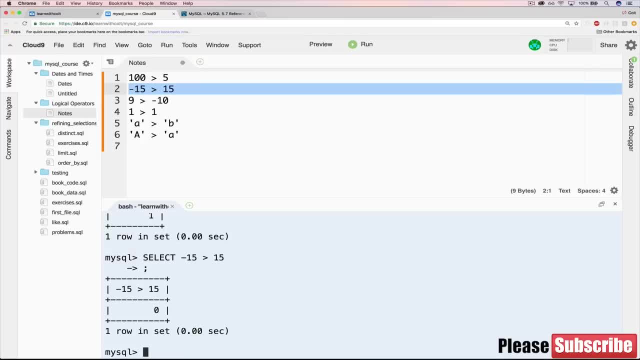 Well, no, I don't think so, And we get 0.. Alright, 9 greater than negative 10.. That seems like it should be true, And it is. What about 1 greater than 1?? Well, I don't think 1 is greater than 1.. 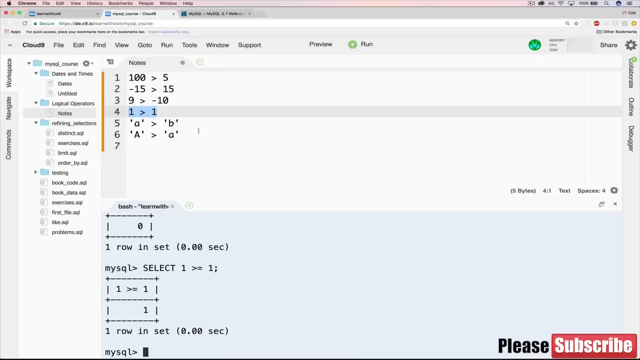 So it's false. However, if there was the equal sign, of course it would be true. Alright, Now these two String comparisons with greater than less than is notorious in all languages for 1 being annoying and confusing and 2 differing radically between. 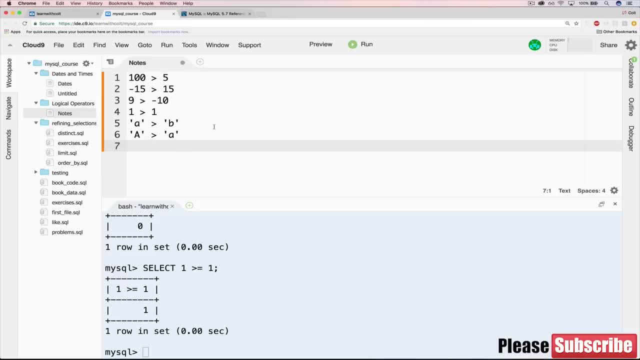 languages. So the advice that I would give to anyone is to just avoid ever having to do anything like this. There are ways around it, But I just wanted to show you what happens. So what do you think Is the lower case? a comes before b. 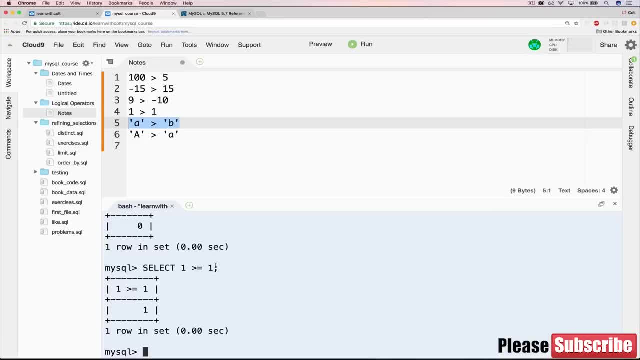 So is it greater than or less than b? And in some languages it is greater than In others. it's less than In MySQL's case. MySQL, if we hit enter, we can see that a is not greater than b, meaning that it's. 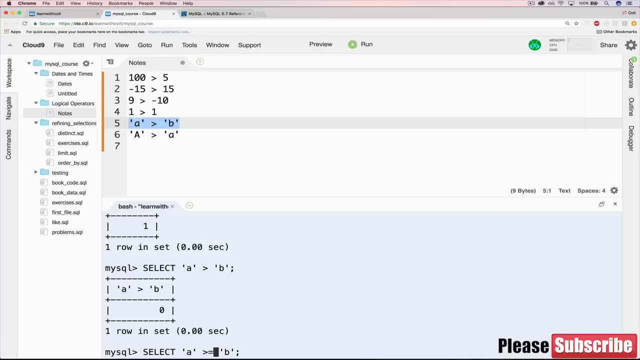 less than b, Although technically that statement is logically wrong because it could be equal to b. But, as you can see, if I add that equal sign, it's still false. So we know, definitely a is less than b. Okay, So that brings us to. 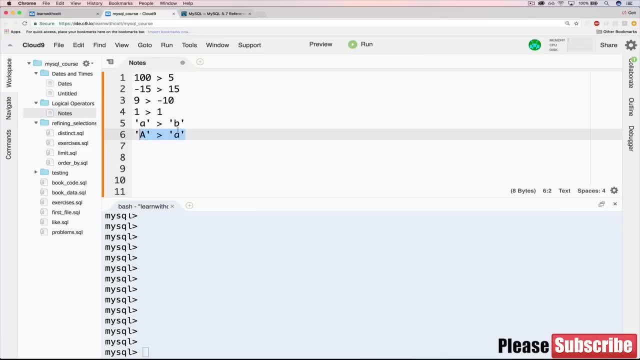 our last one, which is a bit tricky: Upper case a greater than lower case a, And if we run that with a semicolon you'll see that it's false. So upper case a is not greater than lower case a. So then, 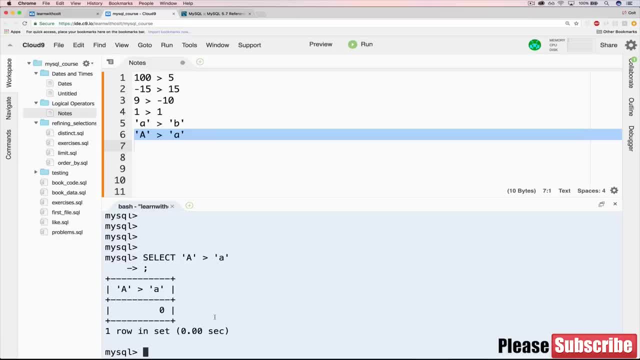 does that mean that it's lower? Does upper case a come before lower case a? And the answer is actually: if we change this just slightly to be greater than or equal to, you'll see now it's true. So that tells us upper case a. 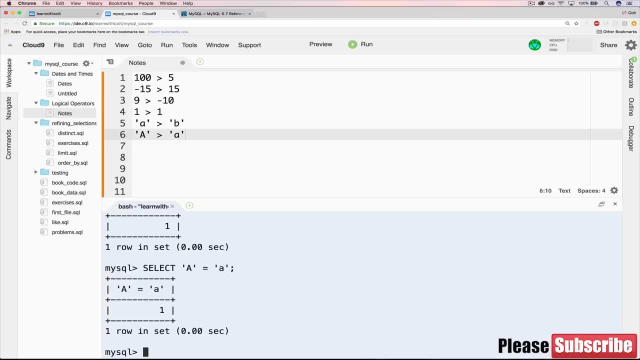 is equivalent to lower case a in MySQL's eyes And we've seen that before. When we do something like- well, let me just type it again: Select author lname, where author lname equals, if we do eggers like this, and of course I add in: 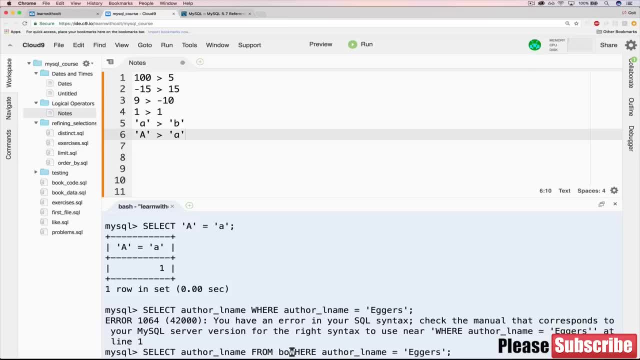 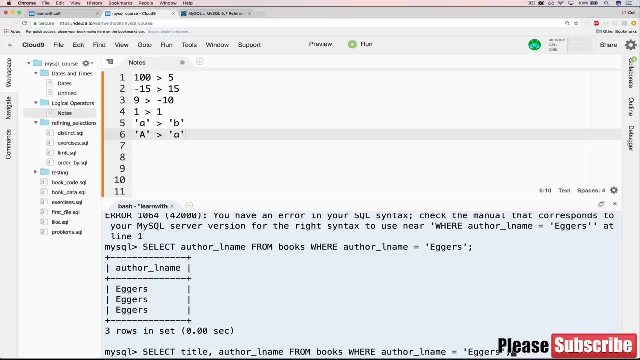 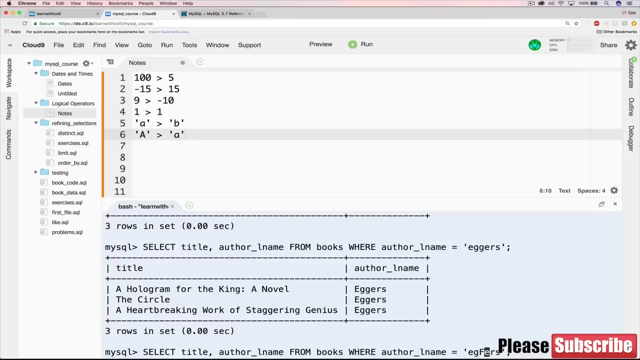 the all important table name from books. So if I do this and let's also do title, just to make it easier to see what's going on, it matches just fine. But I can also do this with lower case e and it works just the same, Or I? 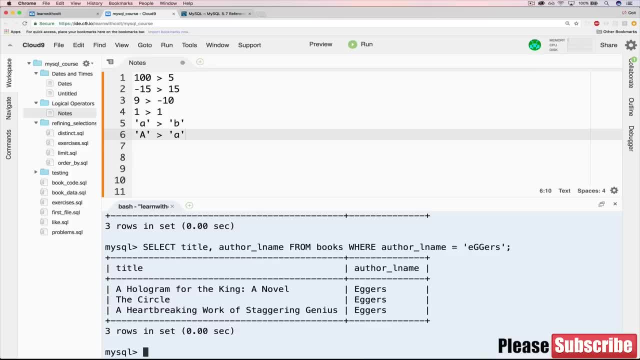 can do eggers like that with two upper case g's. So the way that string comparisons work in MySQL is quite odd, And if you're familiar with other languages, it's very different from pretty much every language I've worked with. So just something worth. 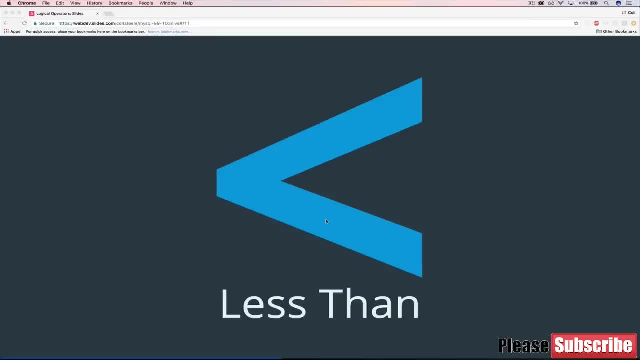 noting That case doesn't actually matter. Alright, so now we're talking about less than We just talked about greater than and greater than or equal to, So this one should be much shorter. In fact, the total time that it will take will be less. 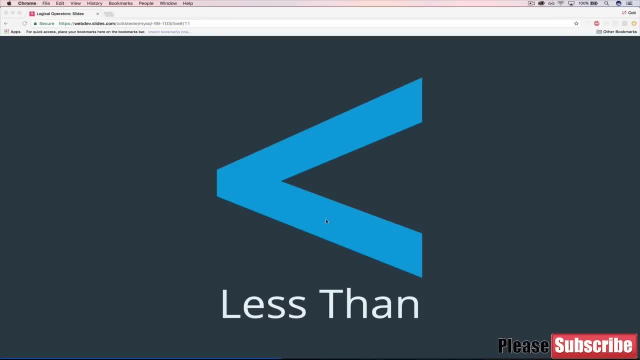 than the previous video. Yeah, So it works the same way, although it does the opposite, If you're familiar. again, it's just the less than bracket- The angle bracket, I think, is what they're called. I just remembered that. So. 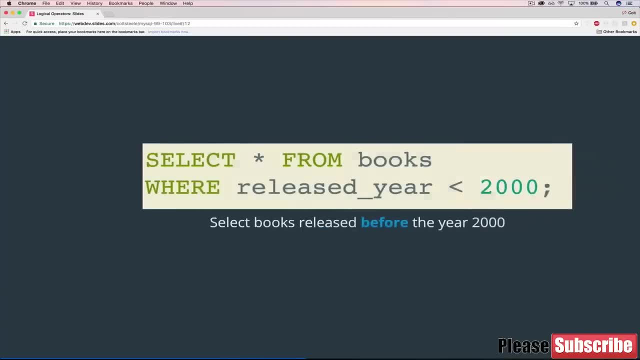 shift and then on most keyboards it's a comma, So we can do things like this. So rather than selecting all books released after 2000,. we just switch it to the less than sign and I'll select star from books where released year is. 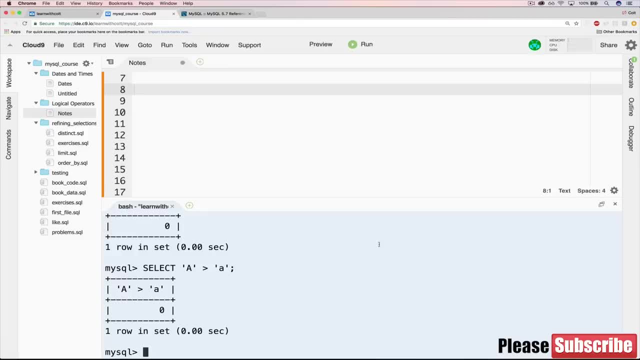 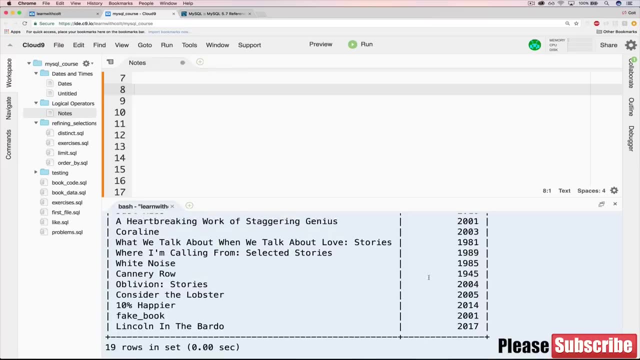 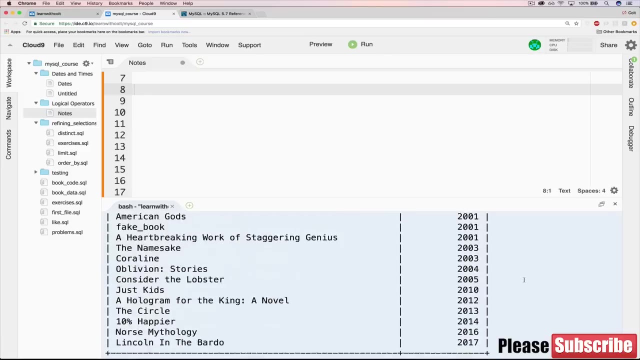 anything below the number 2000.. So if we try that select title and released year from books, If we do all of them, and let's do our order by again Released year, just to make it easier to see where we have missing gaps. 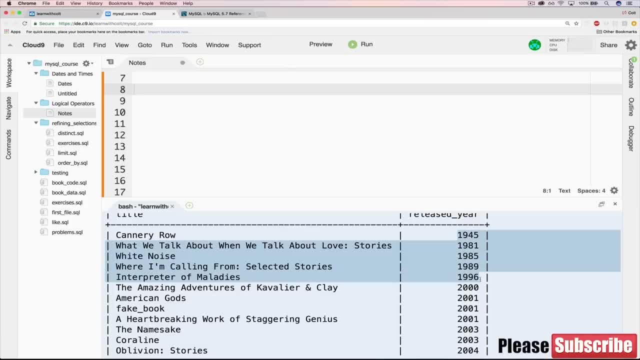 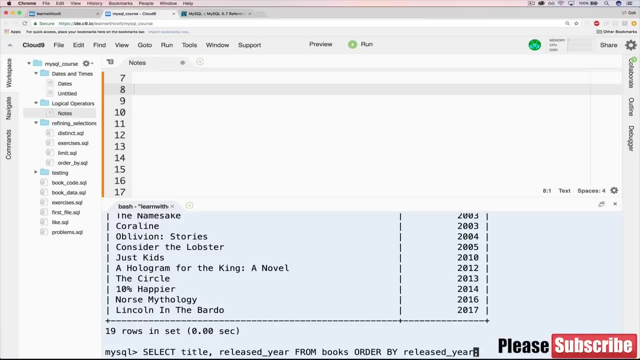 Okay, so we want all of these to disappear, or, excuse me, we want all of these to disappear and we only want to select these five. All we need to do is add in our where released year is less than 2000.. And there we go. 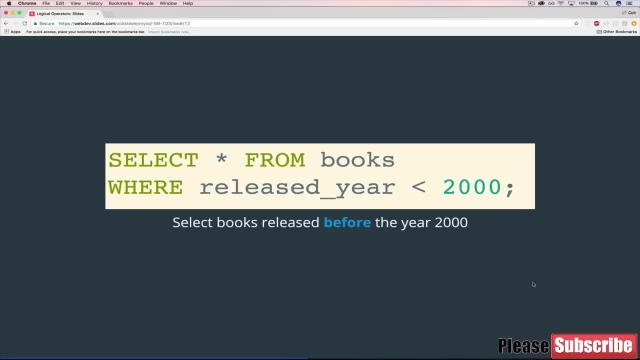 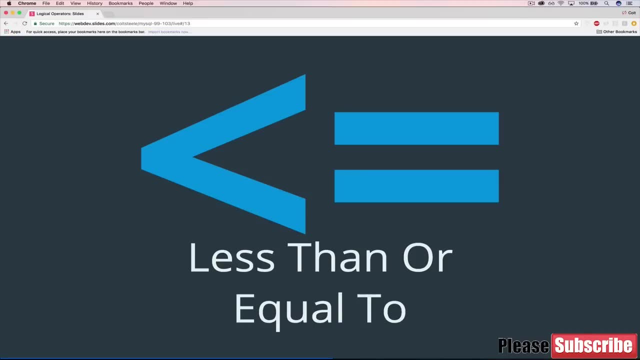 Okay, so that's pretty much all I'll say about it for now. Along with that, of course, we have less than or equal to, which works the same way that greater than well, it doesn't work the same way. It works in the same way that greater. 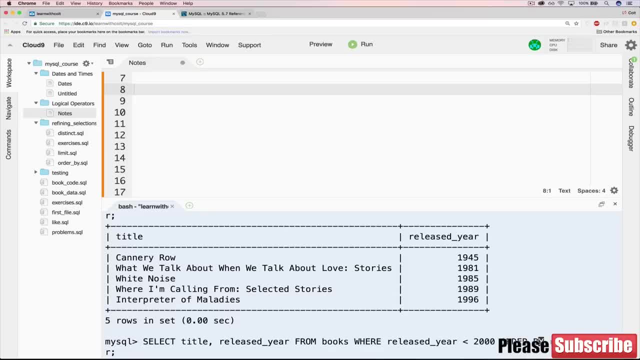 than or equal to does. So if I wanted to include the year 2000, for whatever reason, I just need that equal sign after the less than sign. And now we get the same five books plus the one that was written in 2000,. Amazing Adventures. 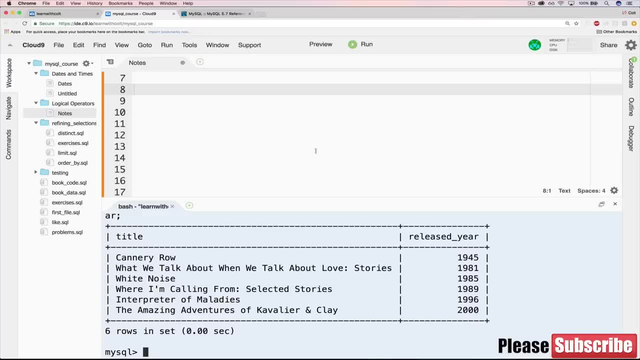 of Cavalier and Clay. That's pretty much it. I will throw up a few exercises here if you want to try evaluating them, And then we're moving on to some more interesting and complex operators. Alright, so I'm back here. I typed. 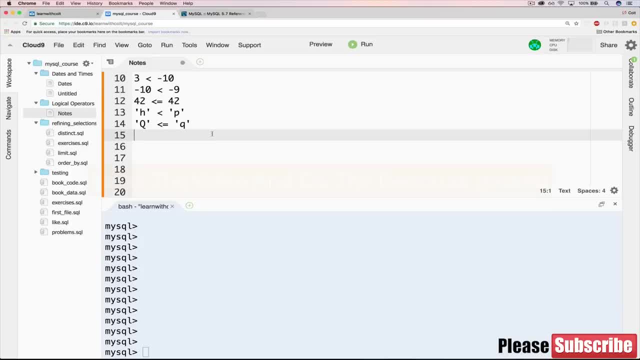 up a couple of quick exercises. Go ahead, try these out. I'll throw up that same graphic again and I'll be back in one second. Okay, I'm back here, So let's go through these quickly. The first one is three. 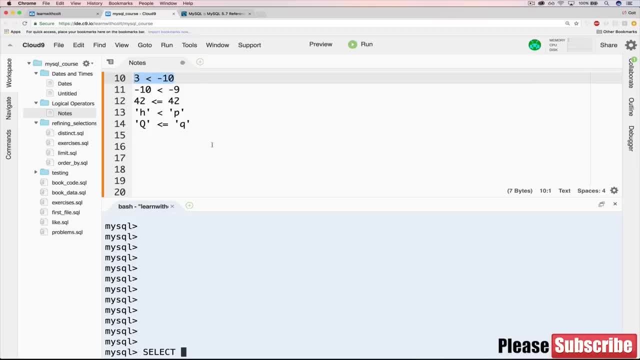 less than negative ten? Well, I don't think so, But let's verify. You can see. zero meaning false, It's not. Is negative ten less than negative nine? Yes, it is, It's lower than negative nine Is forty-two less than. 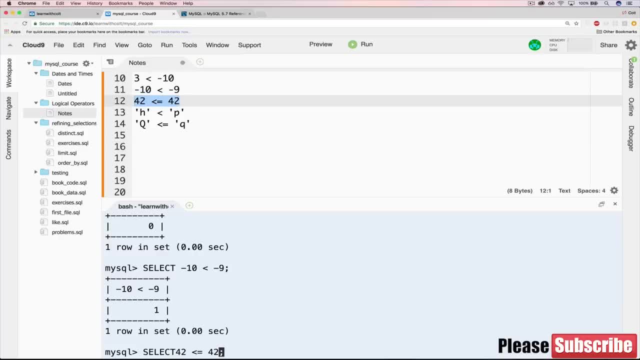 or equal to forty-two, Oop, need to add a space there And, as you would expect, we get. yes, We get one, true, because forty-two is equal to forty-two. And now on to the odd string ones. It's the letter H. 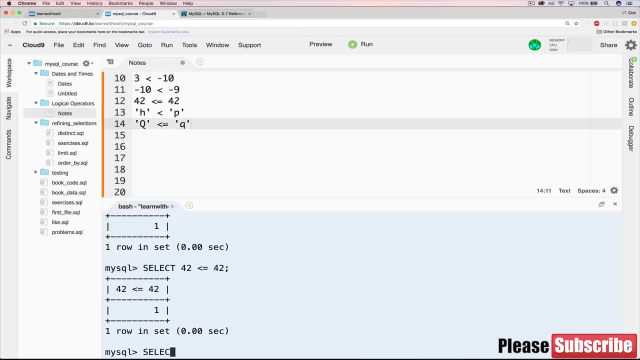 lowercase less than the letter P, also lowercase. And if you remember to the last video, how this works, H comes before P and they're both lowercase. so yes, this should be true And it is Okay. so this final one is uppercase Q. 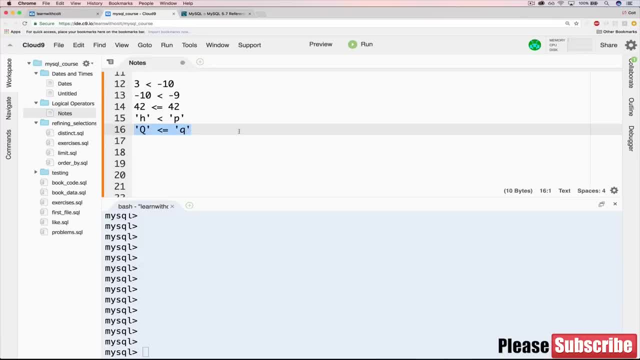 less than or equal to lowercase Q. Well, this should be review from the last video because, remember, that case doesn't matter. So we see that, yes, indeed, it is true, Uppercase Q is less than or equal to lowercase Q. 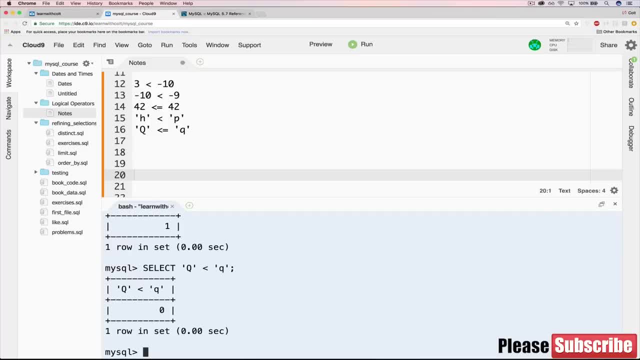 And if we get rid of the equal to this is basically a duplicate of what we just did in the last video. but I just want to hit this home that it is not lower, it's not greater than they are equivalent. Well, 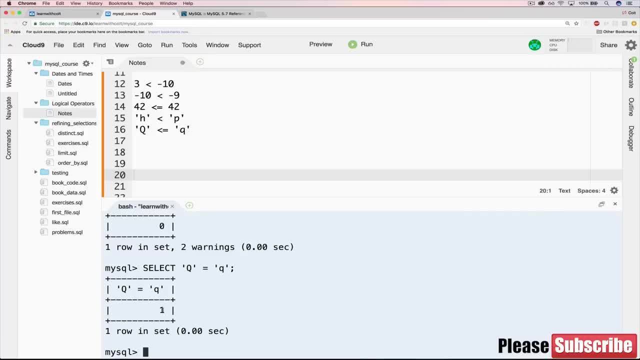 that's a minus sign. There we go. They're equivalent. as you can see. We get true, or one Okay Next up, moving on to much more exciting, much bigger and important logical operators. So in the last video, at the end, I mentioned that we're. 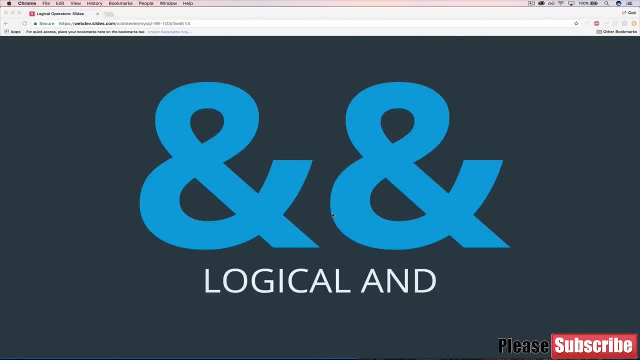 about to move on to bigger and better operators, And this is the first of those. It's called logical AND You'll also see it as just two ampersands, So what it does, it's sort of a step up in operators. 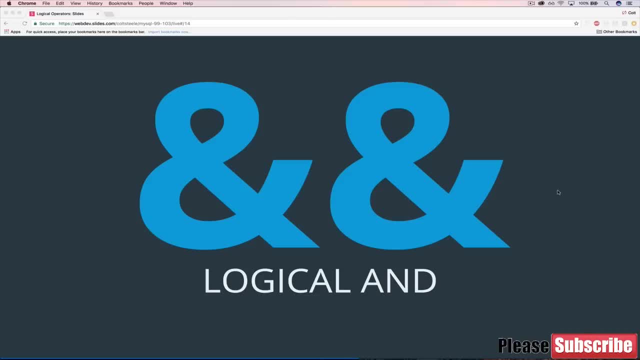 It allows us to actually chain together multiple pieces of logical information, multiple operators together, and basically, it necessitates that all things are true, all conditions are true. Now that sounds like gibberish, so let's put it in practice. let's see what I mean. 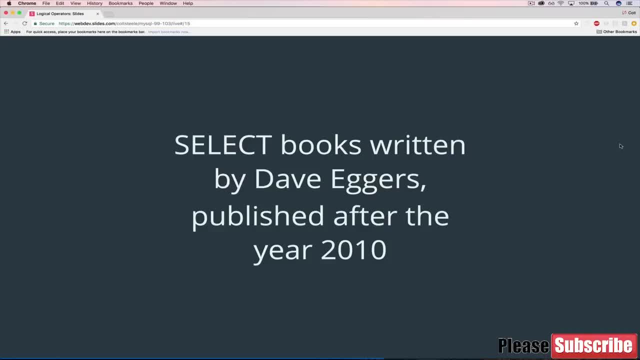 So here's an example. Let's say I wanted to do something like this: Select books written by Dave Eggers that are also published after the year 2010.. So, individually, these are each straightforward tasks. I color coded them to show you. 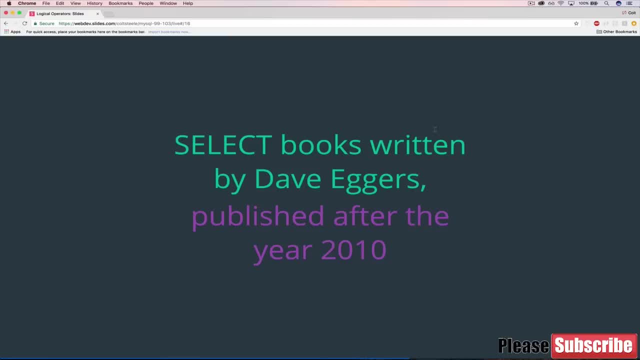 Select books written by Dave Eggers. we know how to do that. We also know how to do select all books published after the year 2010, using greater than what we just saw. However, to put these together, we need to use logical. 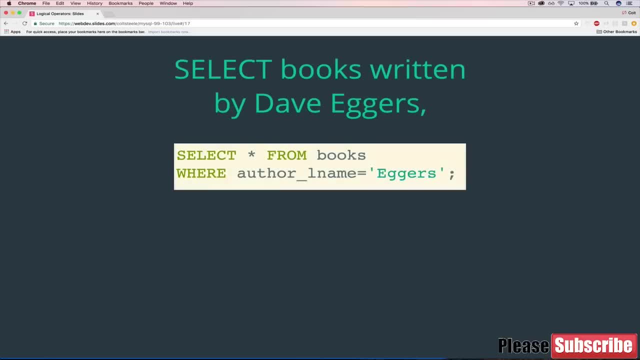 AND So here's the first part: Select books written by Dave Eggers. It would look like this: Select star from books where all author LName equals Eggers, And then to select books published after the year 2010,. it would look like this: 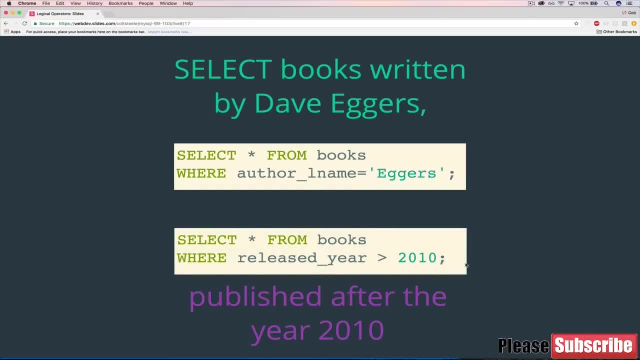 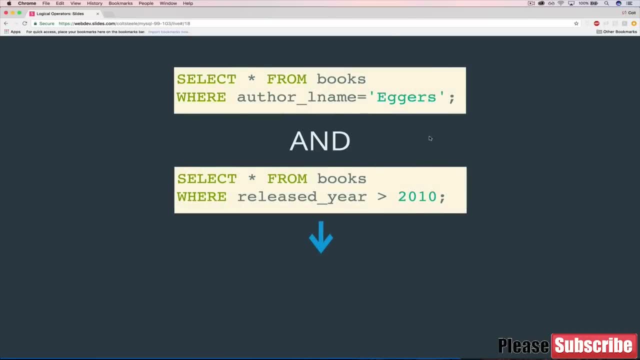 Select star from books where release year is greater than 2010.. So, to put them together, we use AND. Okay, so, as I mentioned, we can either use the word or the text, AND, or two ampersands, And it looks like this: 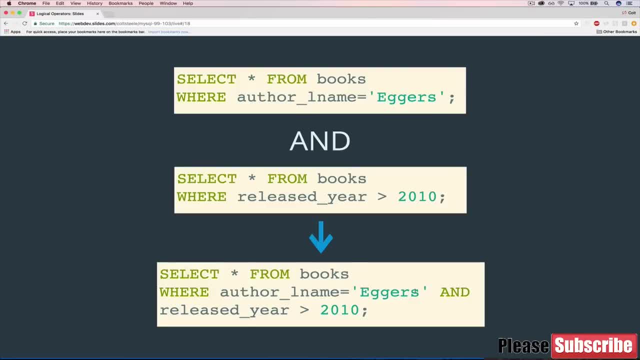 Select star from books where author LName equals Eggers AND released year is greater than 2010.. And that's it. So, basically, we just take the two where clauses and shove them together with the word AND, And what this means is that both parts have to be true in order for 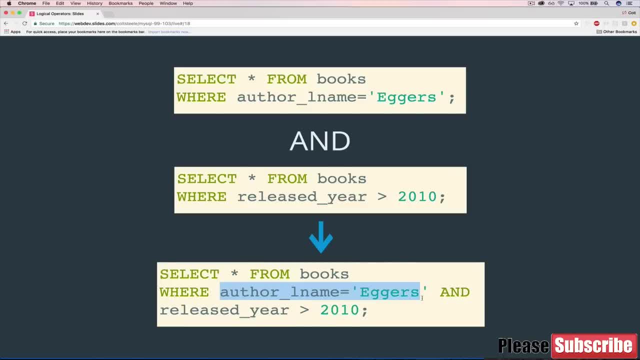 it to be selected, So it will start. it will check: is this author's last name Eggers? If it is, then it will move on and say: okay, AND was it released after 2010?? If it wasn't, then it discards it and it doesn't select it. 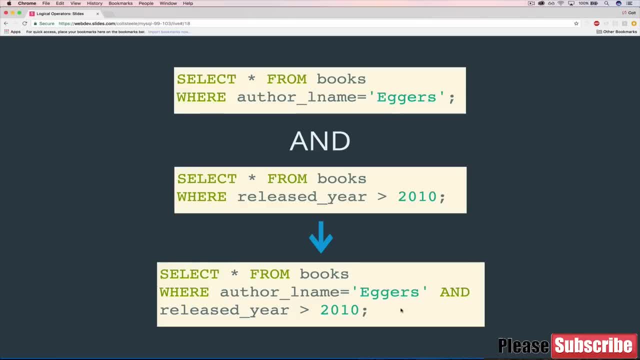 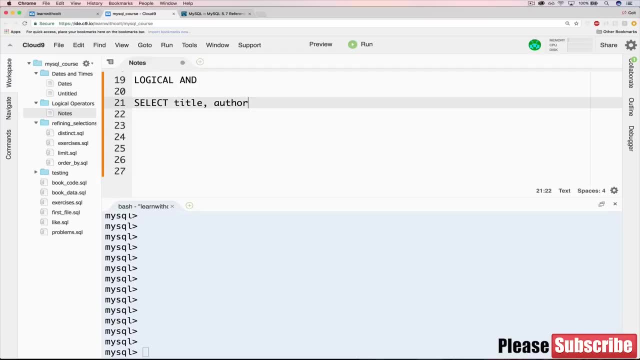 However, if both parts are true, then we see the results. So let's try it. Okay, so let's start off by selecting title, author, LName and released year. And I'm just working in this document, I'm just going to copy and paste in, but I'm just 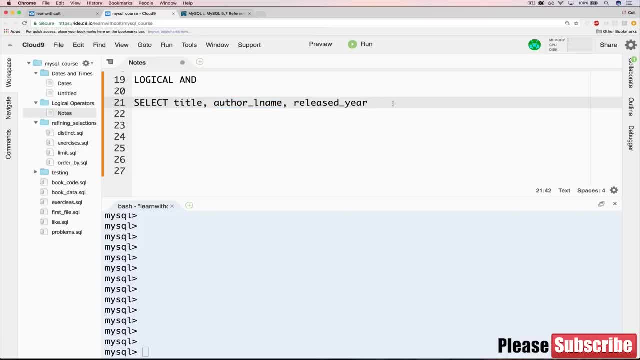 putting a record of it here to make it easier for me to edit as I go through. So select title, author LName and released year from books where- and we're just checking where author LName equals Eggers, just like that. 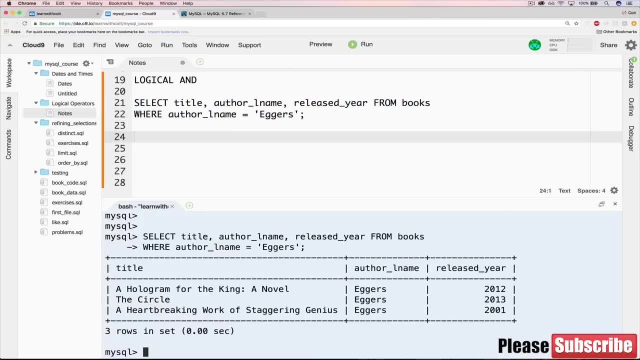 There's semicolon, You can see we have these three: Hologram for the King, The Circle and my favorite heartbreaking work of staggering genius. And then we have released year. So for some reason someone comes into our bookstore and says: you know, I 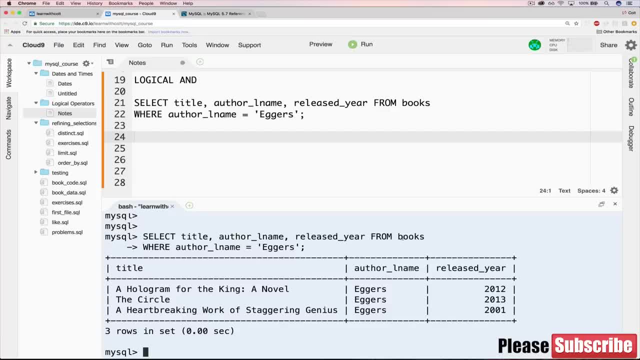 really like Dave Eggers, but I only like his later stuff, which I would disagree with. I think his earlier stuff is better, but let's say someone says that Well then we would do something like select, and I'll actually just copy this: 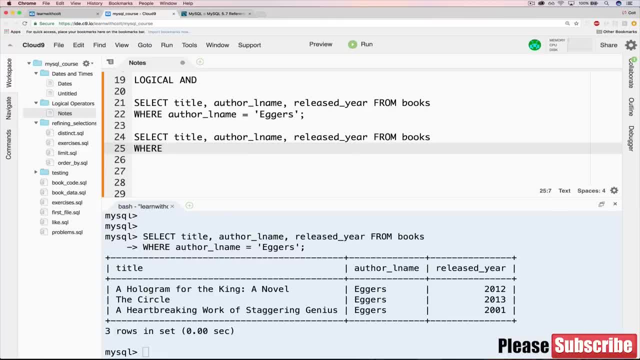 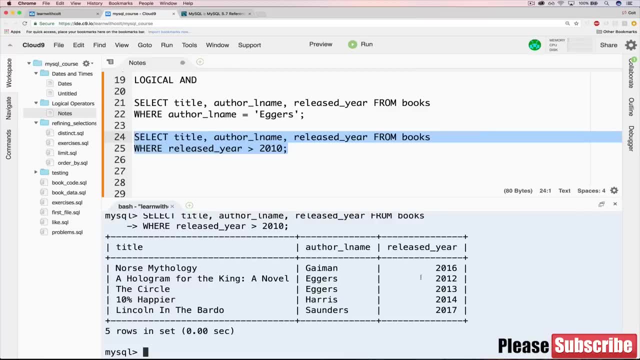 and change the where clause to where released year is greater than 2010,, which we already know how to do. This should be review Now. this gives us all books released after 2010,. and then to combine them is where we use logical. 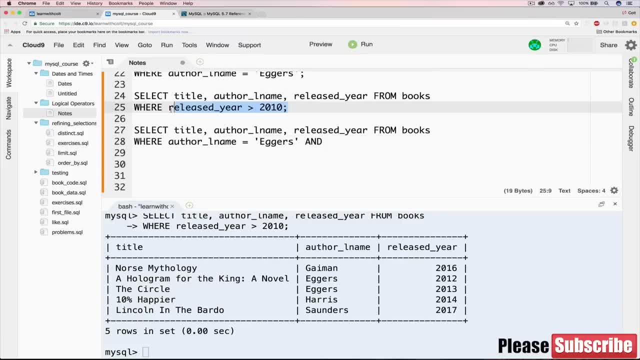 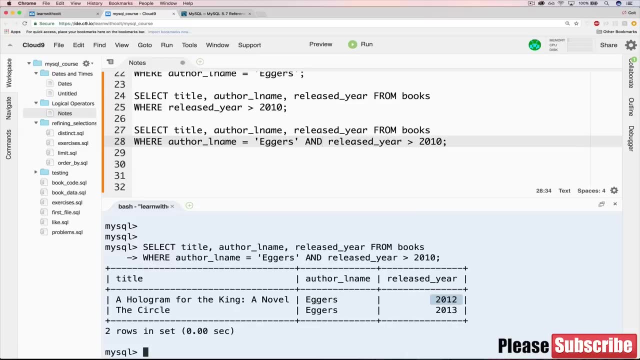 and And released year greater than 2010.. Okay, so let's check that it works. You can see we only get two results because both of these things have to match, So author has to be exactly Eggers- case insensitive. and released year. 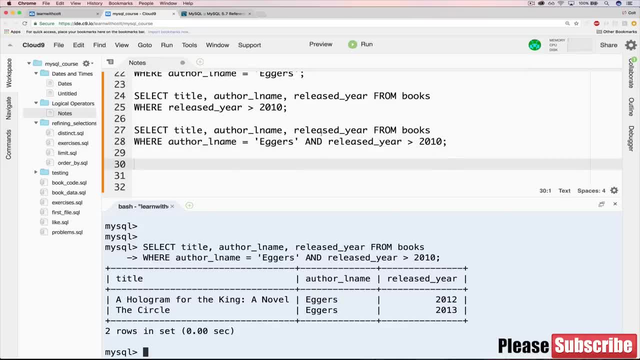 has to be greater than the year 2010.. And just to show you, we can replace this with double ampersands and it works the exact same way. There we go. Okay, so that's the basics of, AND We'll use it all the time. 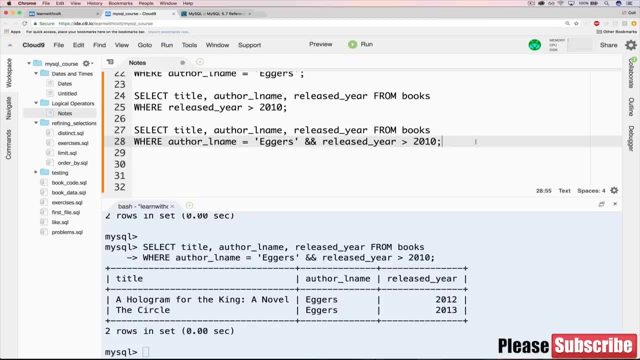 It's important anytime you need to chain together things if you're trying to search based off of two criteria. So a common example might be something like select star from products. Let's say we work in a toy store where brand equals lego. 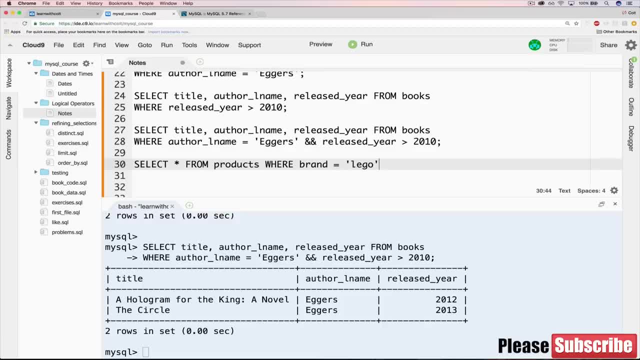 But when you're on a store- an online store- often there's an option that will say show out of stock items or don't show out of stock items. So we could do something behind the scenes, like where brand is lego and in stock. 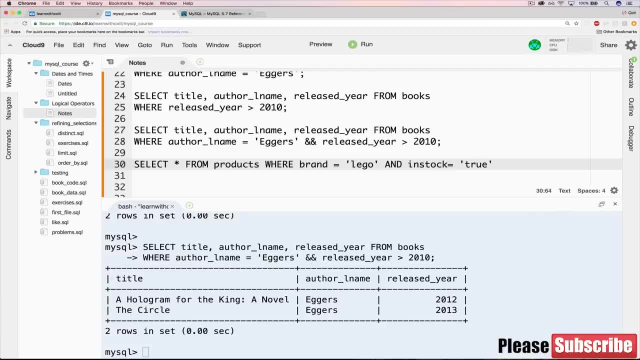 equals true. That way, we wouldn't be showing the customer any lego products that are also out of stock, which is frustrating when you see that. So that's a pretty common use case is when you're working with a value, a Boolean, yes or no. 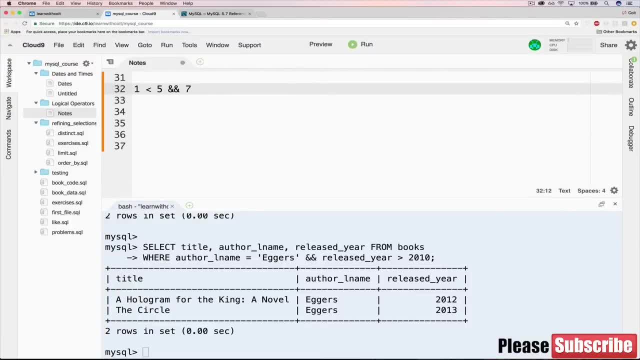 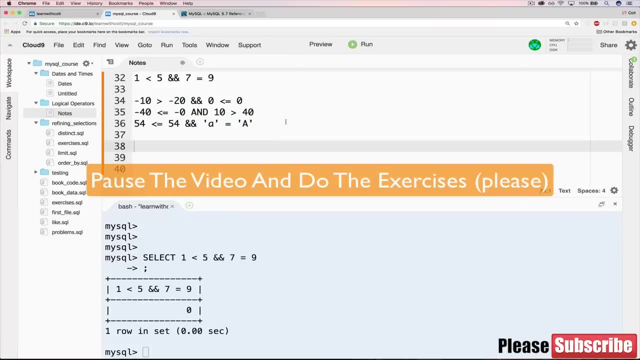 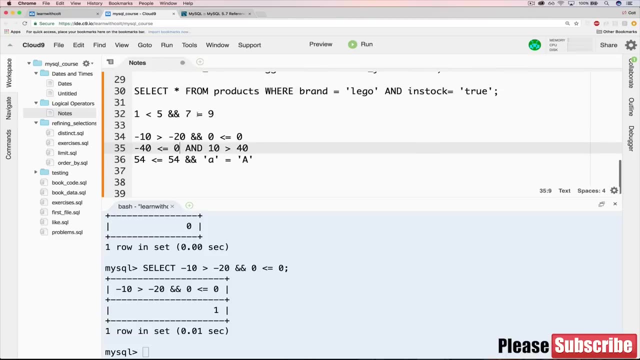 value like in stock or is active user or something like that. Okay, so the last thing that I'll address here is, if we go back to this sort of problem, set things like one less than five, but rather than just doing one on their 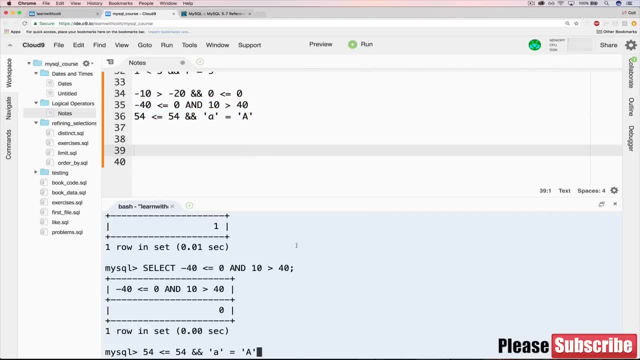 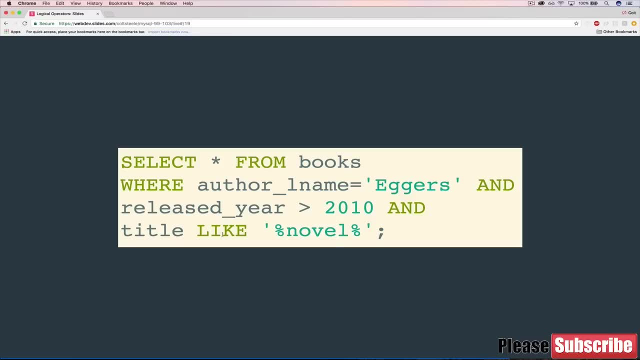 own. I'm going to give you a couple here where we're going to chain them together with and, And I'll give you a first example here. So one greater than five and seven equal to nine. So what does this whole thing evaluate to? 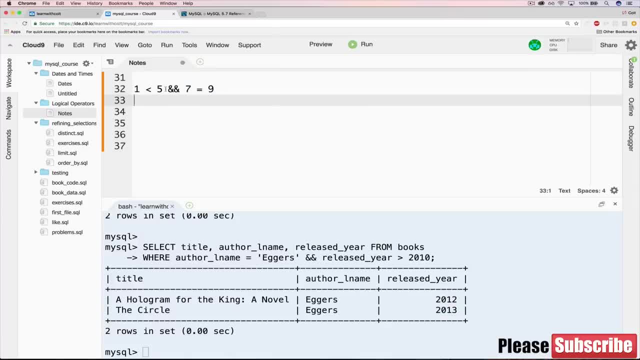 Remember, both sides have to be true, So let's take either side. We'll take this one. Is one less than five? Yes, that is true. Is seven equal to nine? No, that's false and that immediately nullifies or falsifies, excuse me, the. 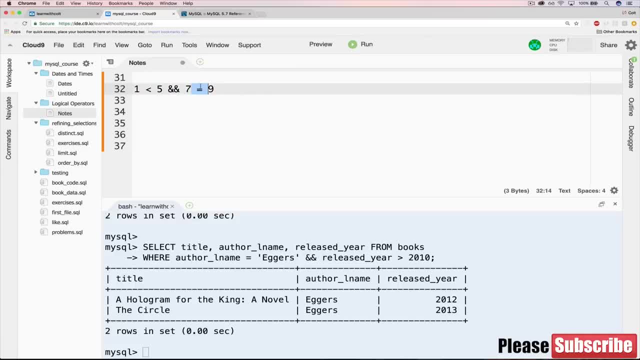 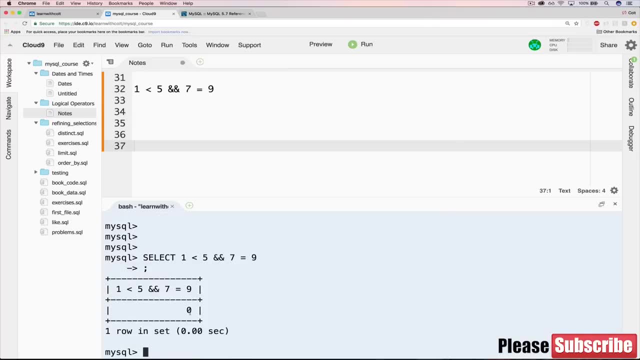 entire thing. Both sides have to be true. Just to double check, let's give it a shot, Select and you can see zero, false, Okay, so, just like before, I'm going to take a moment, fill out a couple of problems and, hopefully, 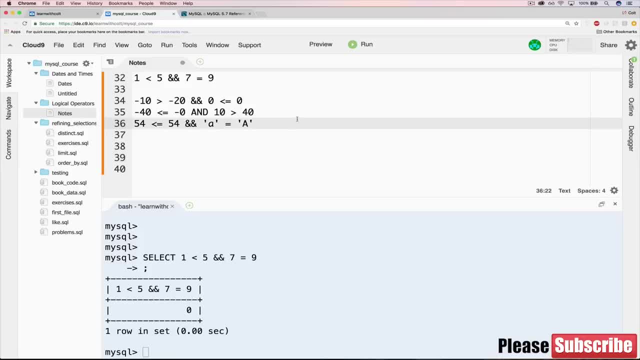 they'll stick around and give them a shot. Alright, I'm back. So I have three simple problems- hopefully simple- that I typed out: Go ahead, give them a shot and I'll be back. Alright, what do you know? I'm back, So let's. 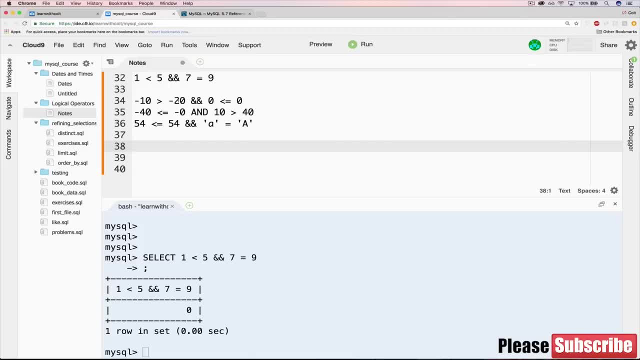 go over these quickly. The first one, Remember: both sides have to be true. So start with the first one: Negative ten greater than negative twenty. Is that true? Yes, It's larger than negative twenty. How about? this Is zero. 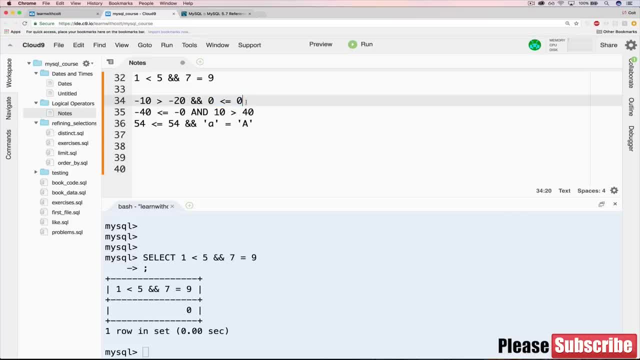 less than or equal to zero. Yes, because zero is equal to zero. Therefore, we have true and true, So this whole thing is true. Let's try it out. Yep, we get one. Okay, moving on, We have is negative forty less than or equal. 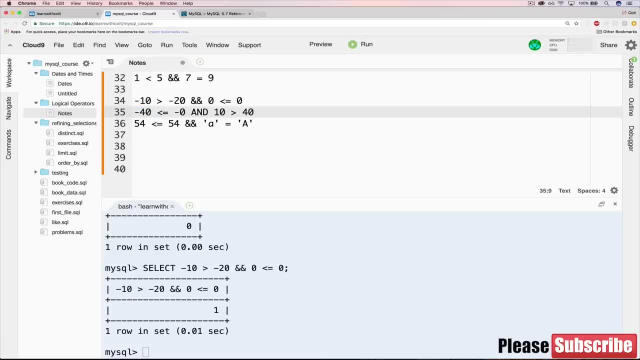 to zero And yes, I know I had a negative sign here. I apologize, That was an accident, That's wrong, So hopefully you didn't spend too much time panicking about that Is negative. forty less than or equal to zero, That's true. 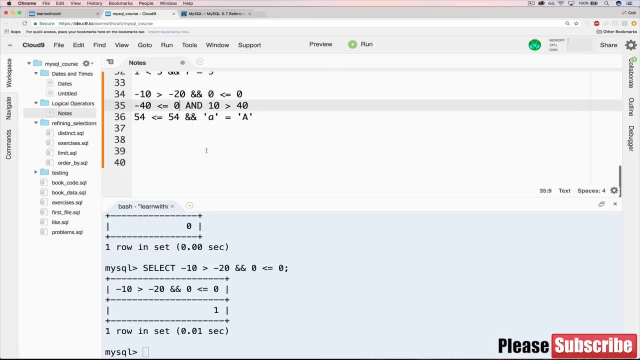 It's smaller than zero- And I used the English version- AND Ten greater than forty. Well, that's actually false, Which makes the whole thing false, unfortunately. So let's try it And we get zero, which means false. 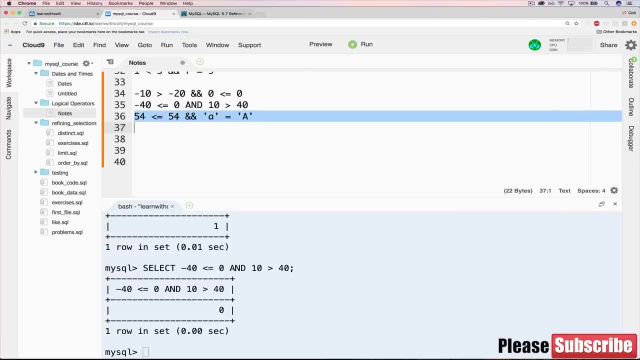 Finally, is fifty-four less than or equal to fifty-four? That's true. Fifty-four is equal to fifty-four And is A equal to A Upper case. Lower case: A equal to upper case. By now you should remember they are equivalent. 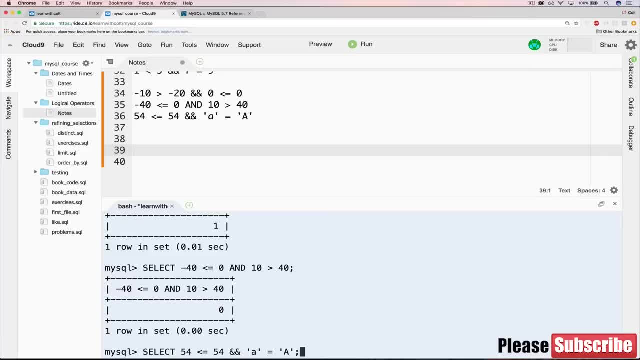 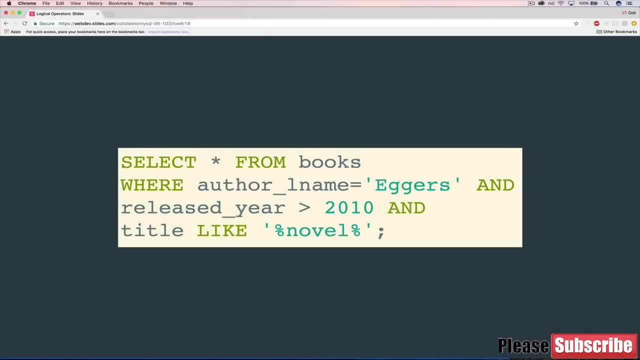 So there's true on both sides And we get true Alright. So the last thing I want to highlight about AND is that we're not limited to just two components, Like we saw here. You know where authorLName is the eggers. 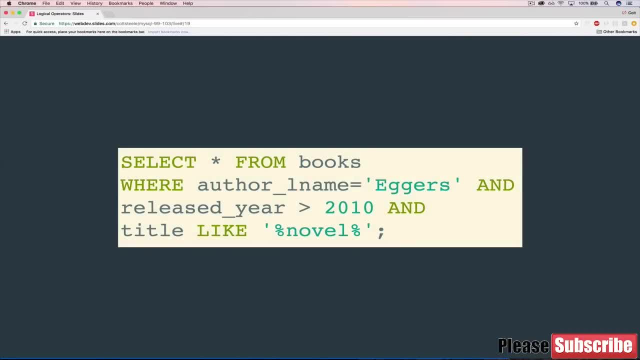 AND releasedYear is greater than twenty-ten. We could do three. We could do twenty if we wanted to. There's probably an upper limit at some point, But typically, if you're working with anything more than really more than three, there are. 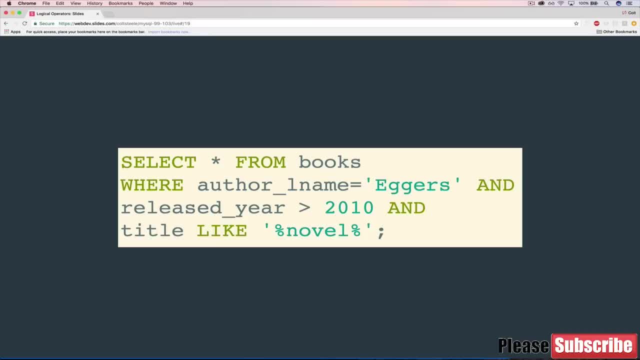 other ways of doing it, Or you may need to change your table structure, which we'll get to once we talk about tables in more depth, when we talk about joins in particular. But in this case, I could do something like this, Where authorLName is eggers. 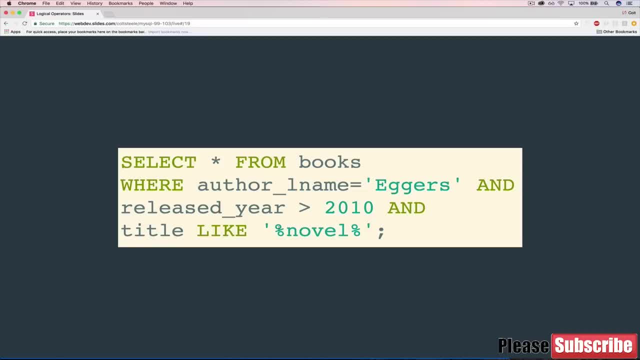 AND releasedYear is twenty-ten AND title contains the word novel. Don't ask why, but let's say we have a needy customer who wants Dave Eggers' book, only likes his later work and wants it to be a novel. And the way that she knows or he knows. 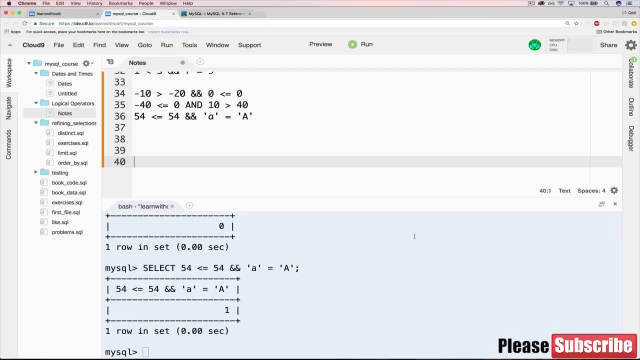 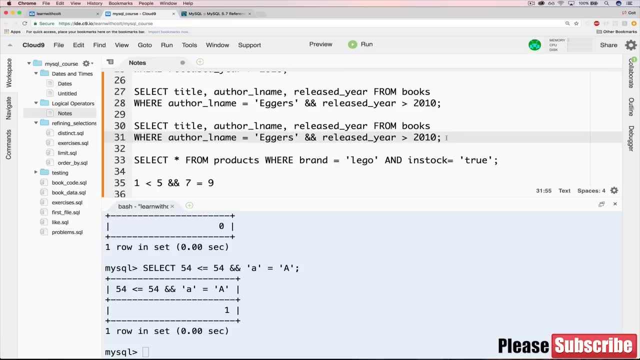 it's a novel, is that it contains the word novel in the title. Well, if we go back to what we had here, Let's just copy this and duplicate it and add another condition, And I'll do them on separate lines now, So I'll do ampersands. 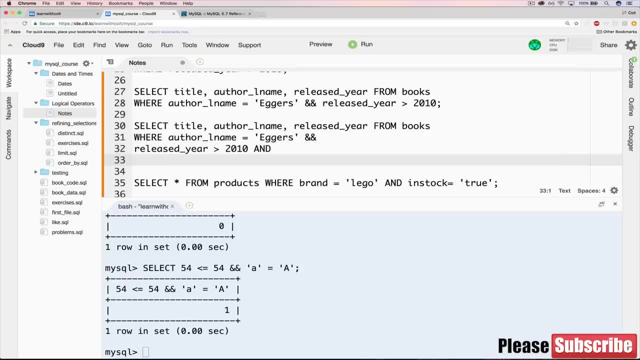 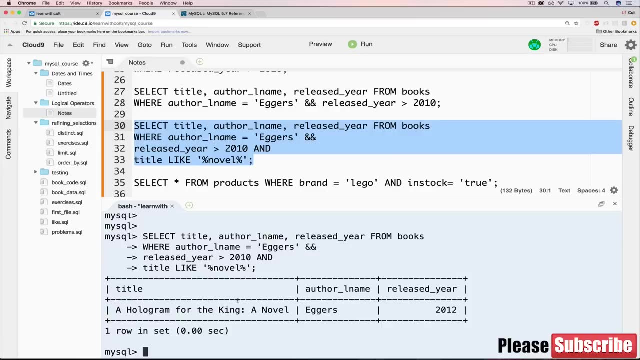 for that one, but then I'll do. AND for the last condition, which is title like: and all that we want is percent novel, percent semicolon. So let's try that, And there we go. We get a hologram for the king, a novel. 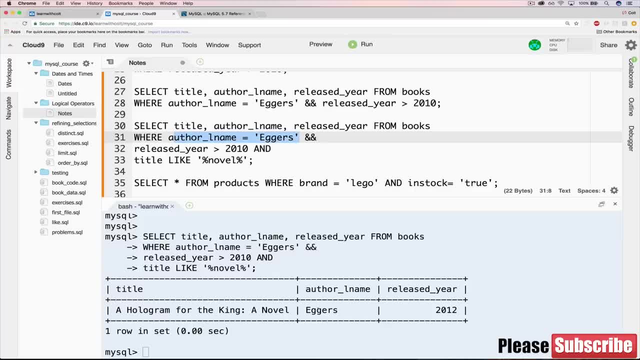 Because, okay, first part: author name is eggers, releasedYear is greater than twenty-ten, twenty-twelve is, and title contains the word novel. So all three are met. So this is the only result we get. So that was just to show you that it's not. 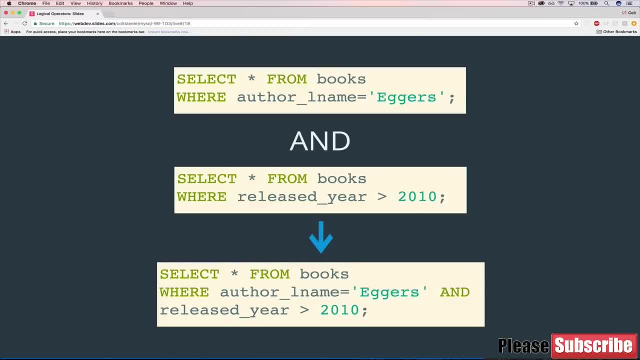 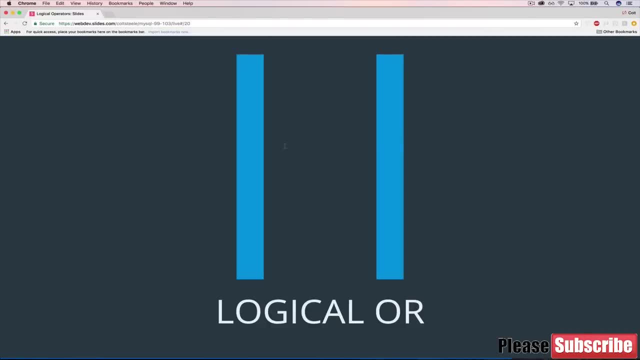 limited to two conditions. Next up, we're going to talk about another kind of sister or brother operator, which is logicalOR. Alright, so we're moving on to logicalOR, which, as I just mentioned, is like the brother or sister to logicalAND. 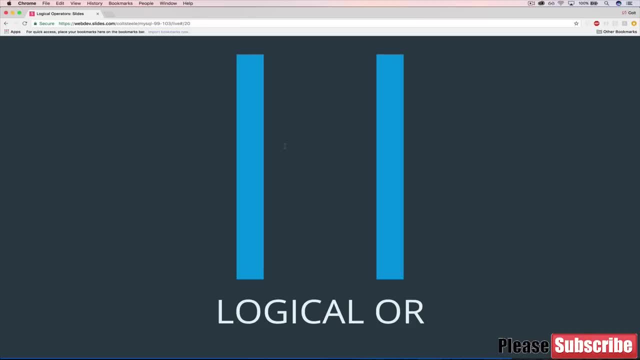 And if you've worked with any programming language, you're most likely familiar with AND AND OR LogicalAND and logicalOR So logicalOR. you can either write out as O-R or just like we could write, A-N-D for AND, or we can use 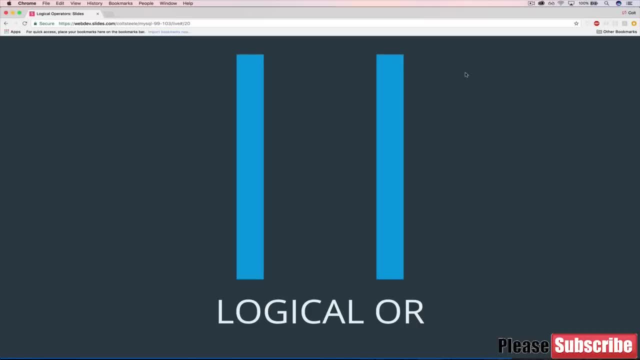 these two pipe symbols. So these are not uppercase I's or L's or ones. They are the pipe character which is usually located above the right return or enter key. You have to hit shift most often to hit it. So it's two of them. 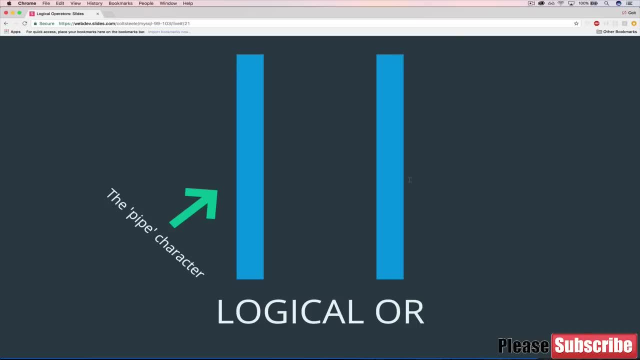 together, just like it was two ampersands for AND. It's just symbols. It's pretty standardized or very standardized across all programming languages that I've worked in: Ampersands for AND, pipes for OR, But you can also use the. 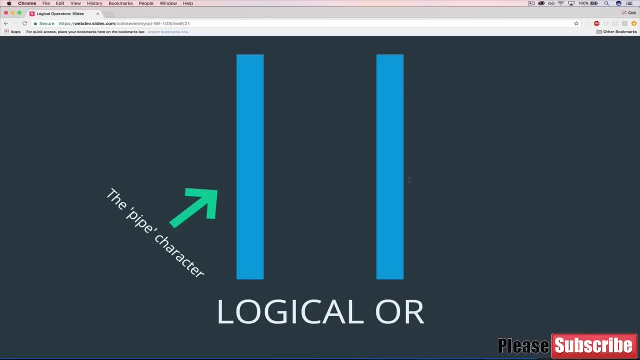 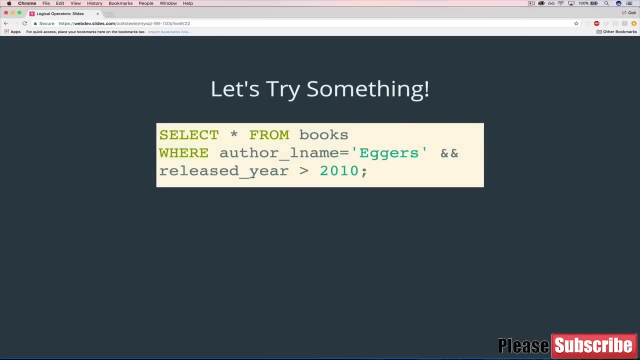 phonetic or the spelled out version O-R. So before we dive into exactly how it works, let's try something. So we had this in the last video. This selects all books written by Dave Eggers released after the year 2010.. 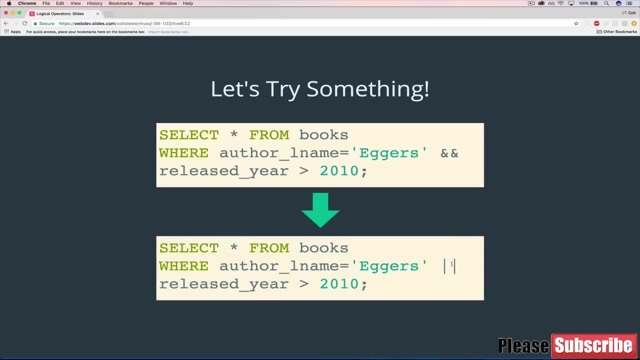 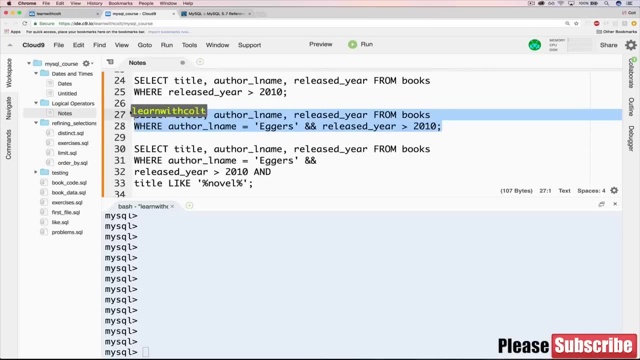 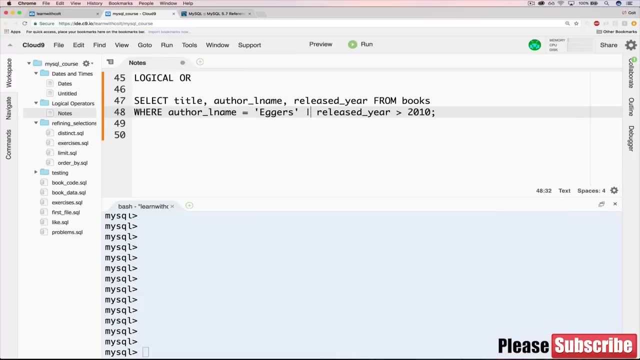 But what if we just change the ampersands to the OR pipes? What do you think will happen first of all? So I'm just going to copy this, so we don't have to type this all again And just change the ampersands here. 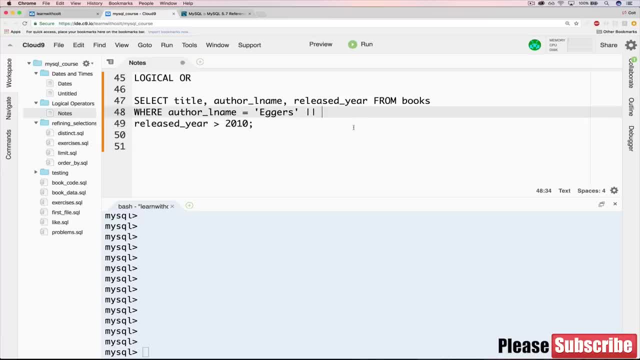 to OR And I'll hit return so it's clearer what's happening. So if we read this, if you just say the word OR here, it makes a bit more sense. Select title and author name and released year. from books where author name is Eggers or. 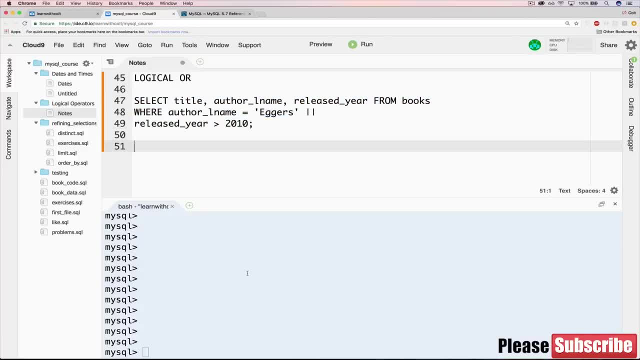 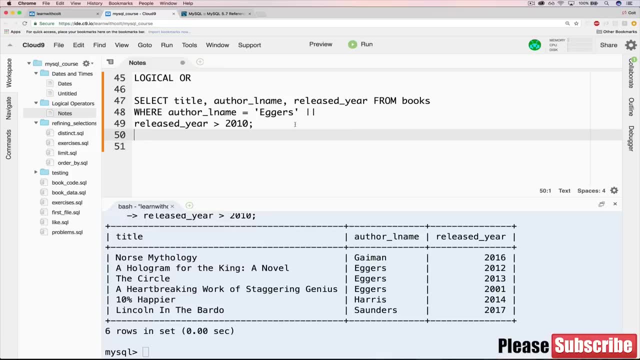 released year is greater than 2010.. So if we run it, what we'll get is all books written by Dave Eggers and all books where released year is greater than 2010.. So rather than both sides of this having to be true, just if either side is, 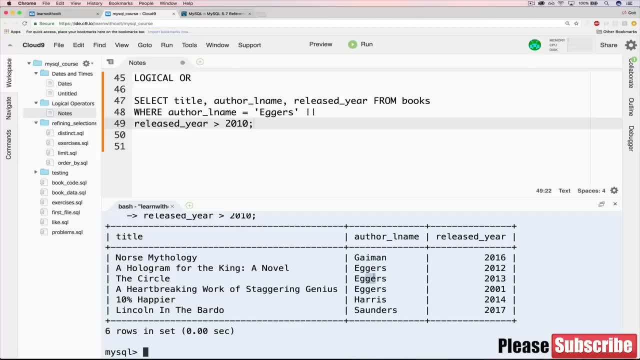 true, we'll get the data. So we get all the books by Eggers, including this one, A Heartbreaking Work, A Staggering Genius, which came before 2010.. But then we move on to the second part, which MySQL. 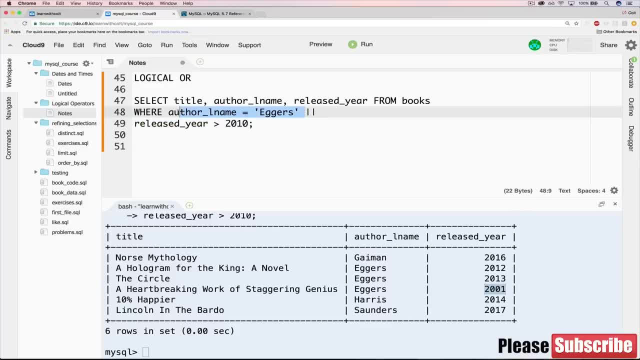 selected all books that were released after 2010,. regardless of the author name. So it's a way for us to specify two things, either of which we want to be true, or both. So, in the case of A Hologram for the King, 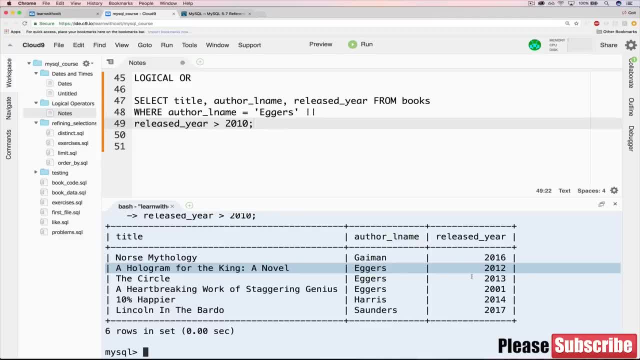 it is both written by Dave Eggers and it was released after 2010.. Or same thing with the circle here, But 10% Happier, for instance, was only this part was true. released year is greater than 2010 because author L name is. 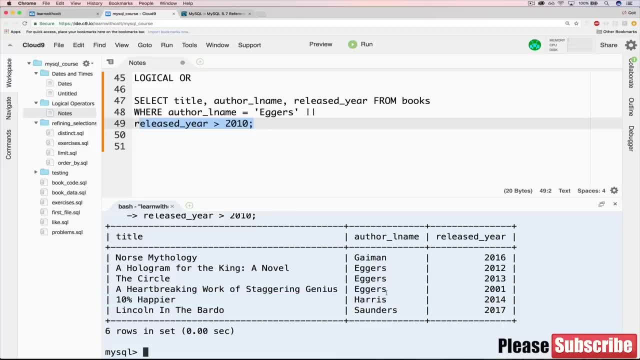 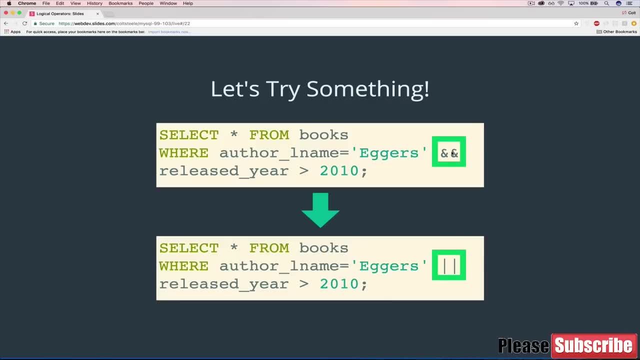 Harris, or Saunders in this case, or Gaiman. Okay, So again that symbol. right there I forgot. I made this nice little slide, this animation. that change of symbol is very, very important. It changes the meaning entirely from the. 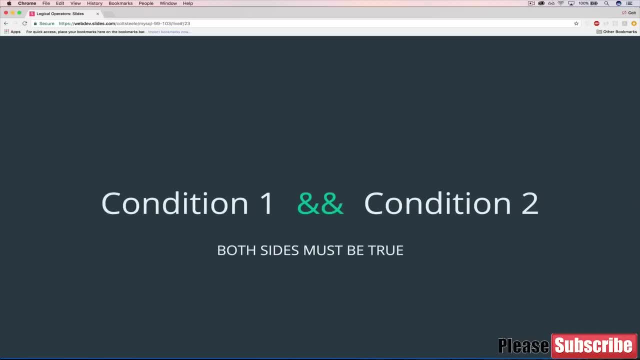 statement. So if we have two conditions with an ampersand between them, or three or any number of conditions with ampersands, it means that both sides must be true in order for the whole thing to be true. as we've seen already, 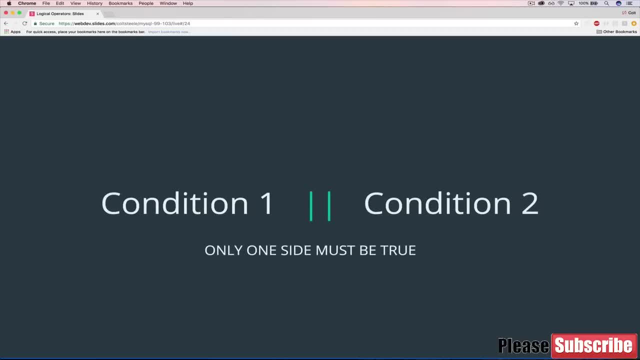 However, with the OR operator it means only one side must be true for the whole thing to be true, or both sides can be true as well, And I know that's a bit odd to talk about in this way, without actual examples. So if we hop over again, 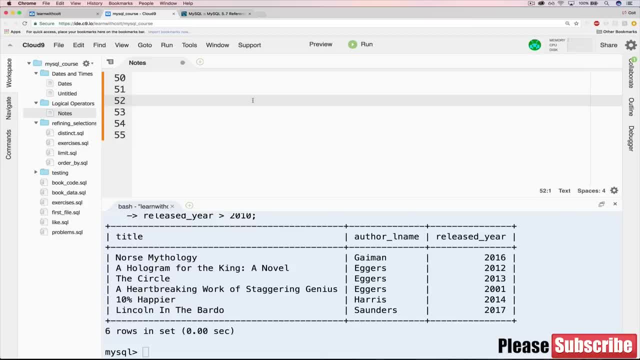 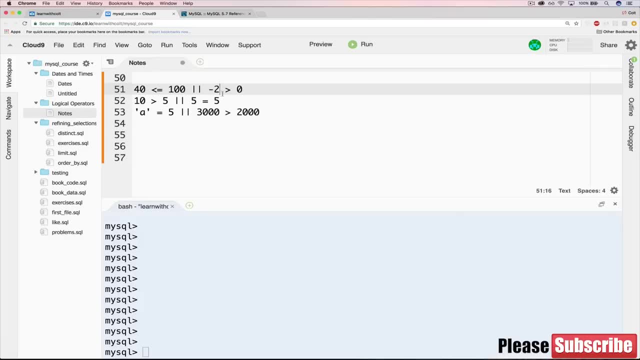 I'm going to do the same thing I've been doing the last couple videos: I'm going to type up a few example exercises and then we'll go over solutions. Okay, so I'm back here. I've got three, just three this time- that all use. 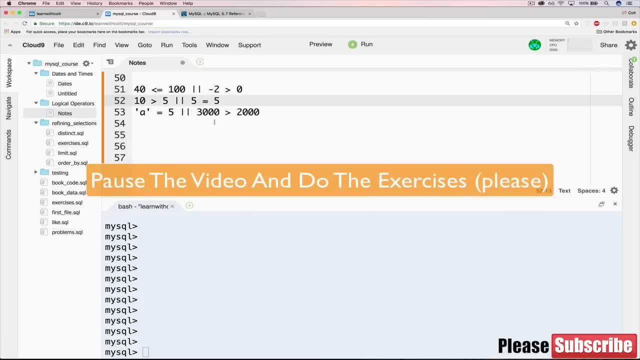 logical, OR So try them out, and then I'll be right back with a solution. And I'm back already, Okay. so first one here: 40 less than or equal to 100.. Well, that part's true. 40 is less than 100, so 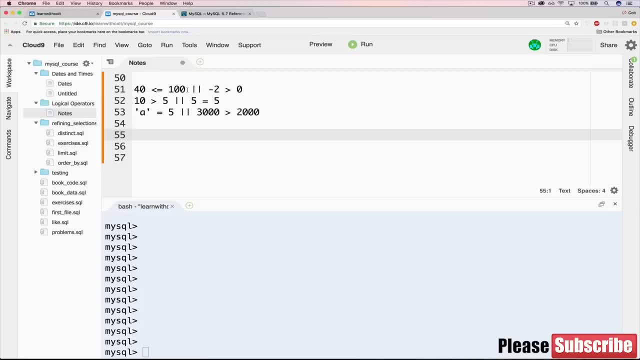 it doesn't matter what's over here. This whole thing is true because we only need one half to be true. It happens that negative 2 is not greater than 0, but that's irrelevant, because the left side is true. Moving on to this one, 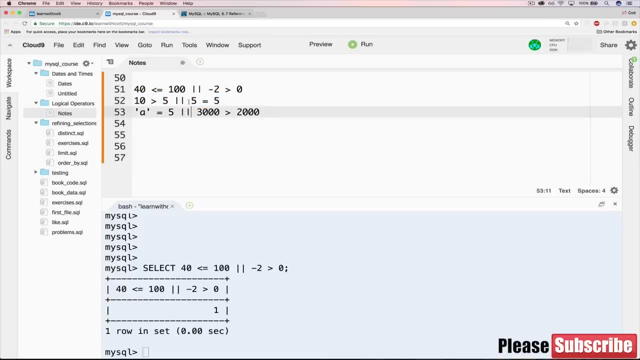 10 greater than 5, is that true? Yes, So it doesn't matter what's on the right side, but that happens to also be true. so the whole thing is true. So we get 1.. And this last one bit of a. 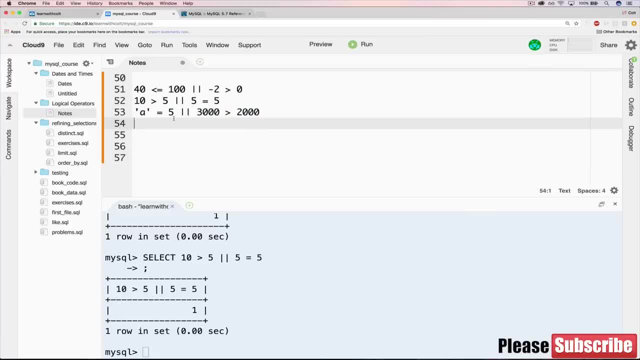 curveball. is the letter A equal to the number 5?? Well, that's not true. However, this side says 3000 is greater than 2000,. that is true. so the whole thing is true. As we can see, we get 1 for true. 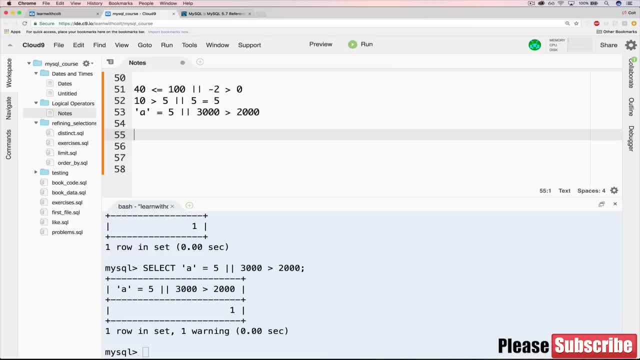 Okay, last thing before I forget. just like with AND, we can chain OR together as many times as we want, so it doesn't have to be something like this. So if I go back to this example, select title: author: L name released here from books. 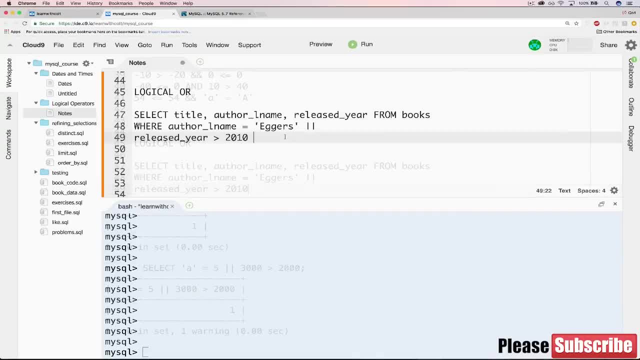 where author name is Eggers, OR released here is greater than 2010.. So let's try adding an OR here- and I'll spell it out this time- and let's say: not only do we care or do we want to select things written by 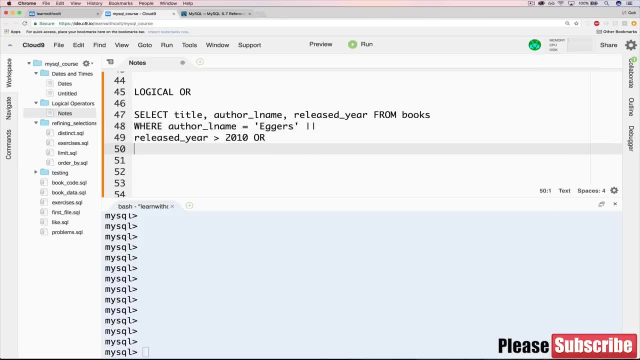 Eggers. OR released here greater than 2010,. we'll also add another OR, which is stock quantity is greater than 100.. So books that we have a lot of stock in as well, And let's also print stock quantity, Just like that. 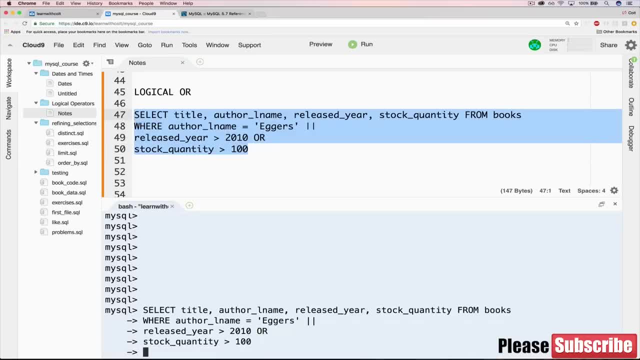 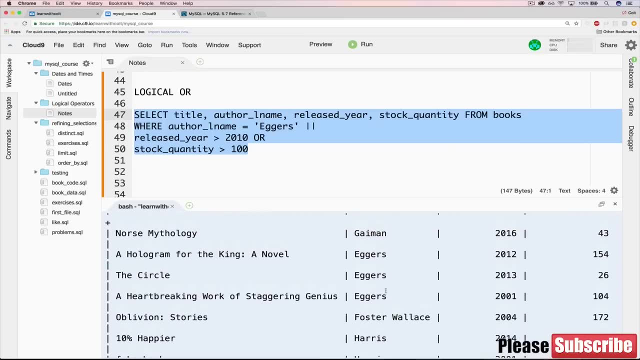 Let's copy this whole thing, paste it semicolon, and if we look see it makes a slight difference, because we also get this David Foster Wallace story collection in here, which was written in 2004,, which normally wouldn't make the cut with our 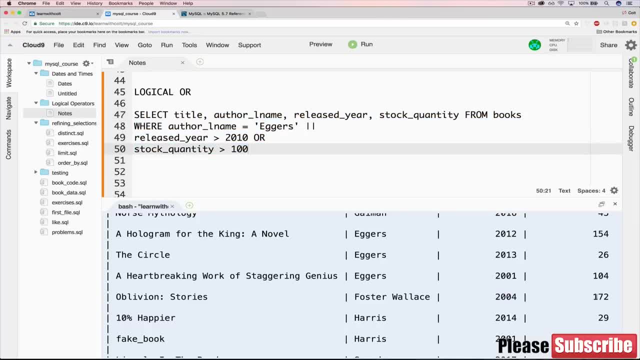 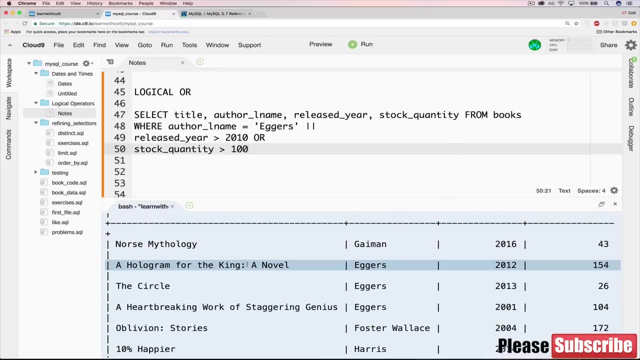 previous version, but because we added stock quantity greater than 100, it's in here Because stock quantity is greater than 172.. So for some of these, for instance, a hologram for the king, all three parts are true. It's written by Eggers. it's released. 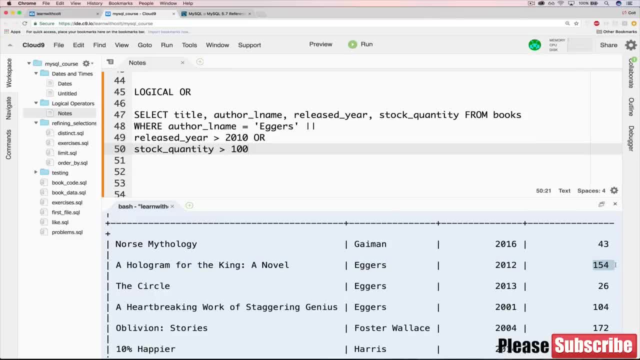 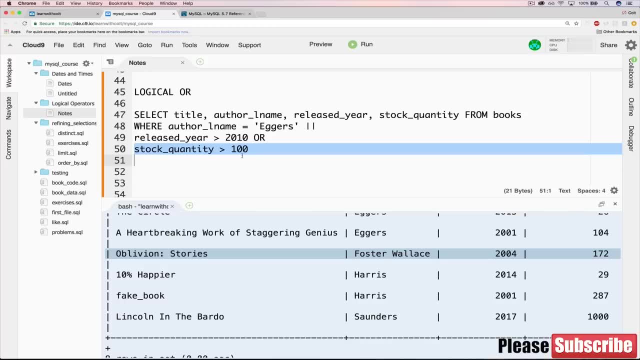 after 2010, and it has more than 100 copies in stock. But then, like for David Foster, Wallace and Oblivion, only one part is true, the last part. So it just goes to show you that only one component, even if we have three. 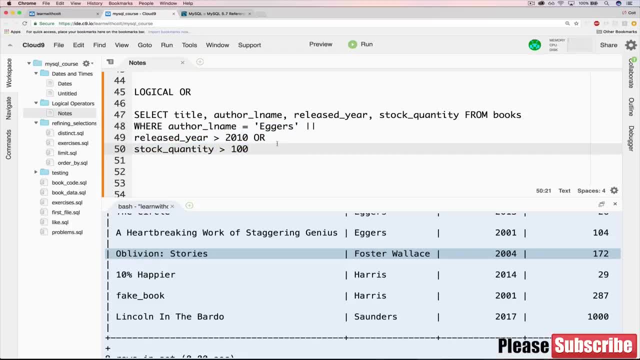 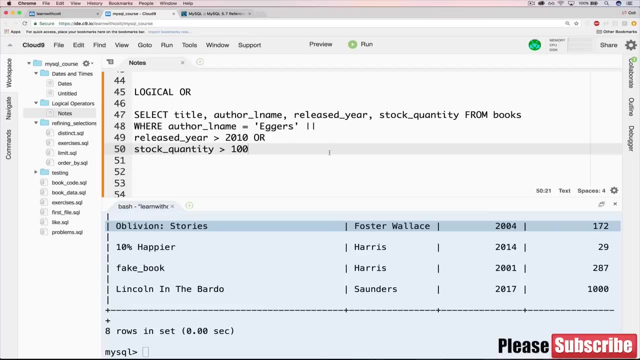 different conditions. only one part has to be true for the entire thing to be true and for it to be selected and spit back to us. Okay, so that's logical. OR One thing that I will point out that I know you're probably dying to: 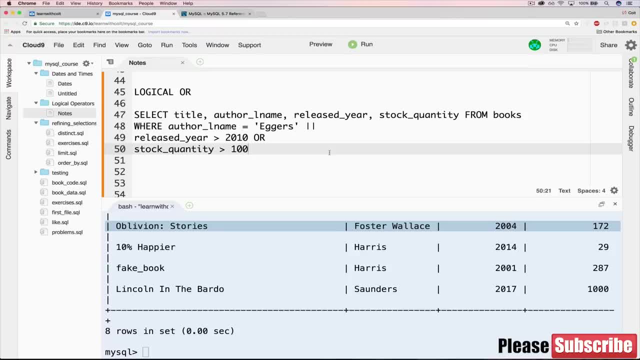 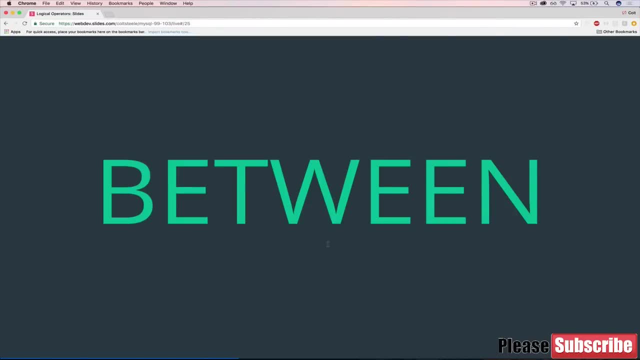 get on with this video, but you can combine OR and AND, and we'll see how to do that in a little bit. So, moving right along, our next operator we'll take a look at is called BETWEEN, And BETWEEN is pretty straightforward. It allows: 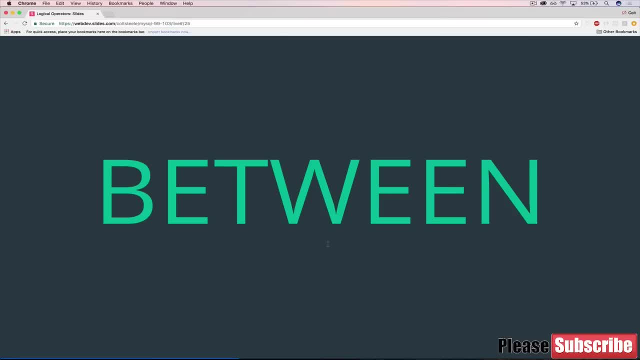 us to select things based off of two values in upper and lower range. So I can say: I want to find all people who have a birthday between April 20th of 2017 and April 22nd of 2017.. Or I want to find all books. 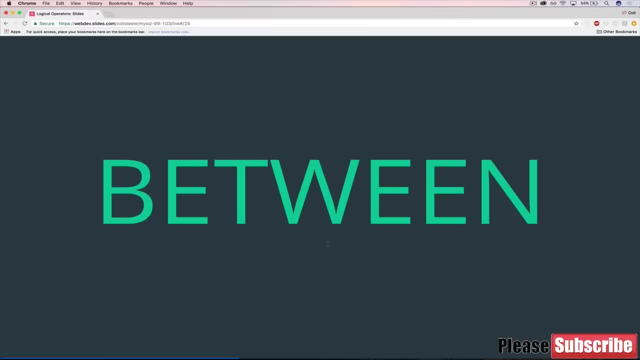 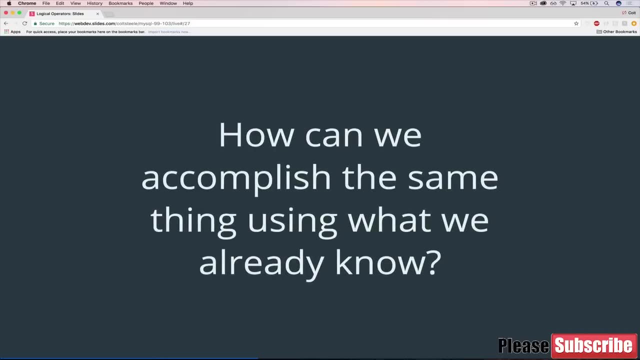 that have page counts between 100 and 500 pages, So we actually can do this already using what you know. So, before I show you BETWEEN, how can we accomplish the same thing using the tools that we already have, Things that we learned in this section. 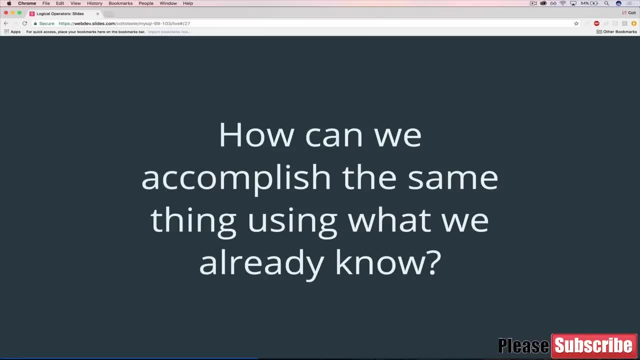 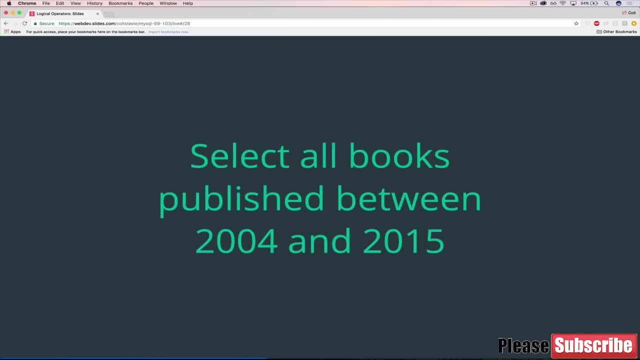 already, Because if you take a moment to think about what being BETWEEN two values actually means, it's really just a combination of GREATERTHEN and LESSTHEN. So how do we combine two different conditions? Well, LOGICAL, AND So let's try an example. 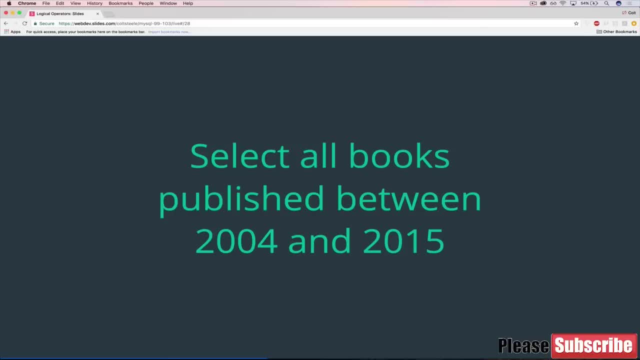 again, just to reiterate, if I wasn't clear, We're doing it without the new BETWEEN operator. We haven't seen that yet. We're doing it the longer way, If you will So, select all books published between the years 2004 and 2015.. 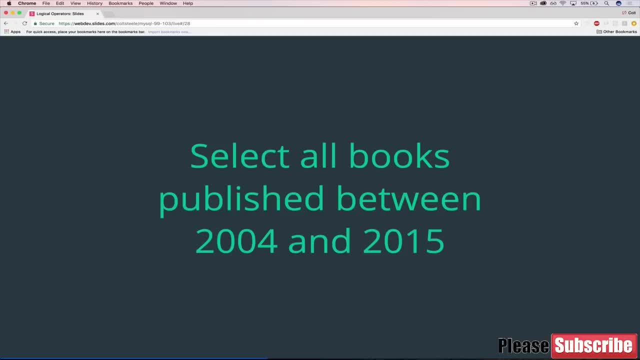 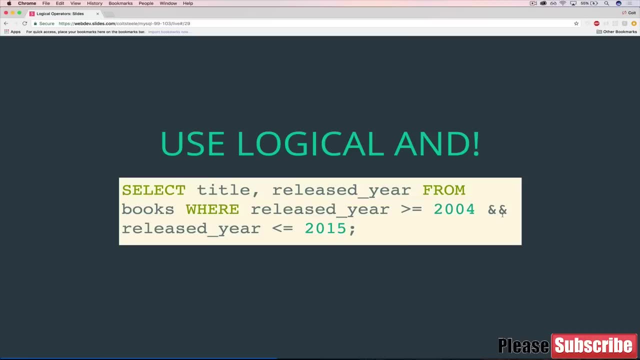 And that includes 2004 and 2015,, just to be clear. So to do that we use LOGICAL AND to join together two different conditions, two components. So select title and released year. blah, blah, blah, that doesn't matter- from books. 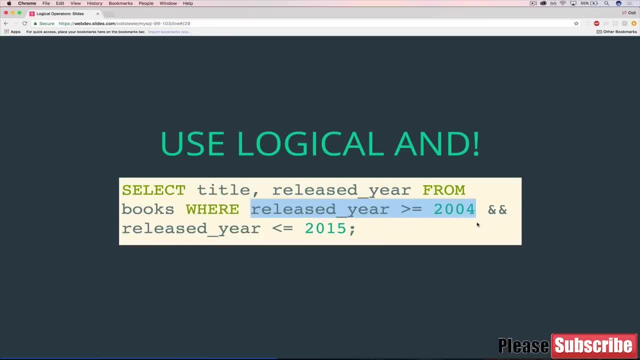 where released year is greater than or equal to 2004 and released year is less than or equal to 2015.. So both parts of that have to be true, meaning that whatever the book is that's selected, or all of the books that are selected. 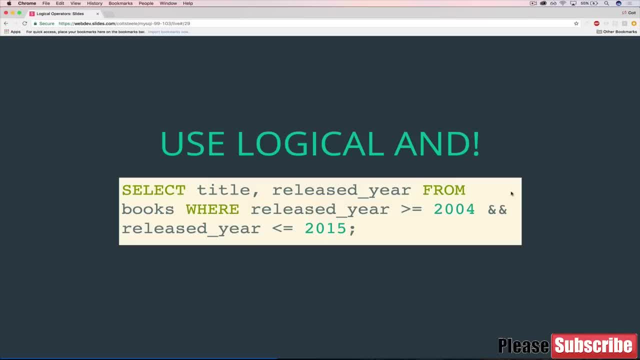 are somewhere between 2004,, including 2004,, and 2015,, including 2015.. So I won't make you watch me type this whole thing, I'm just going to paste it over here. But let's start off by just doing. 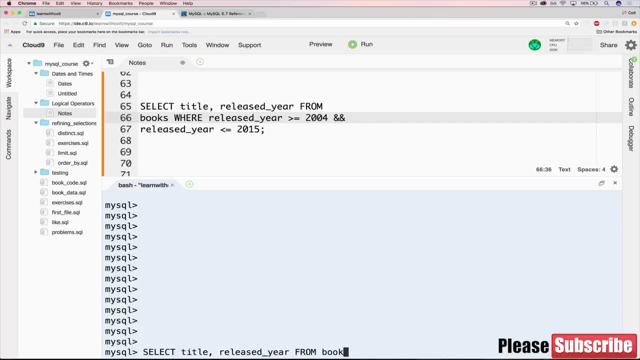 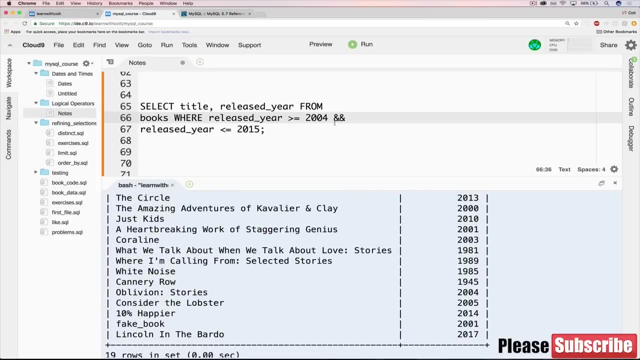 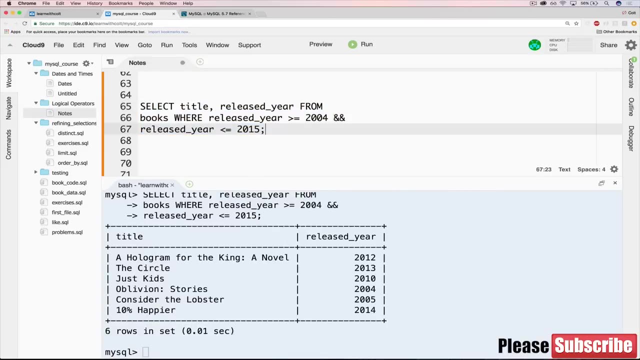 select title and released year from books and just check. we know this, but just to verify that there are things outside that range. And now, if we paste in using the ampersand, ampersand and operator, which of course could also be: 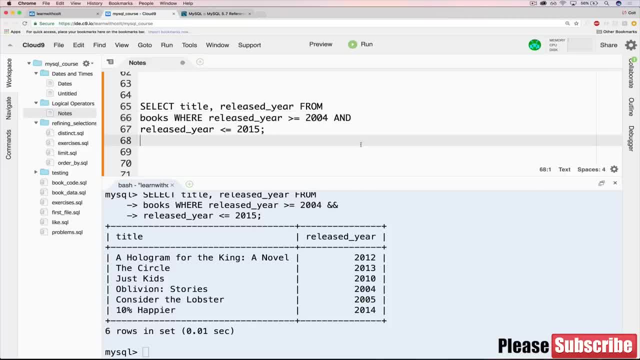 written this way, if I could type correctly, you'll see that we get things that are between 2004 and 2015,. and we know that it's inclusive, as you can see, because 2004 is here And if we 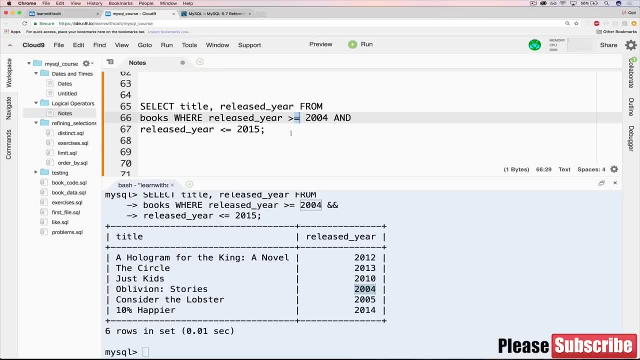 hadn't included that equal sign, then it would not be there. Okay, so really, what I'm trying to show you is that you don't need a fancy between operator to accomplish this. you can just do it using good old fashioned logic, using greater than and less than. 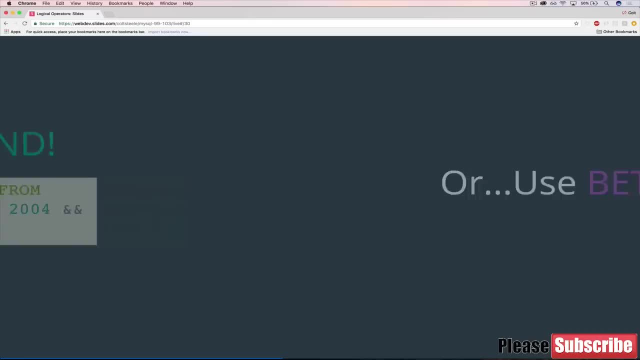 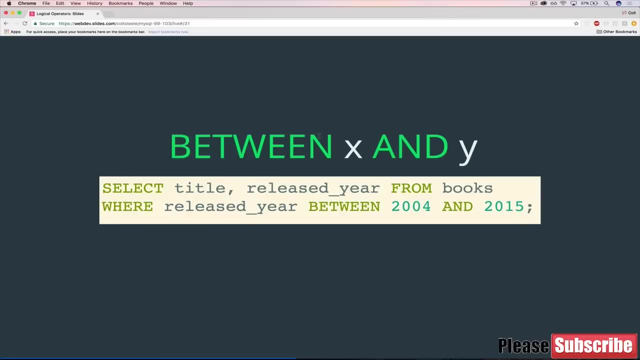 and a logical and. However, there is an operator between. that will make it easier. So it looks like this. The syntax is between: and then some value and some other value. This and here. just I get it. it could be confusing when we also have 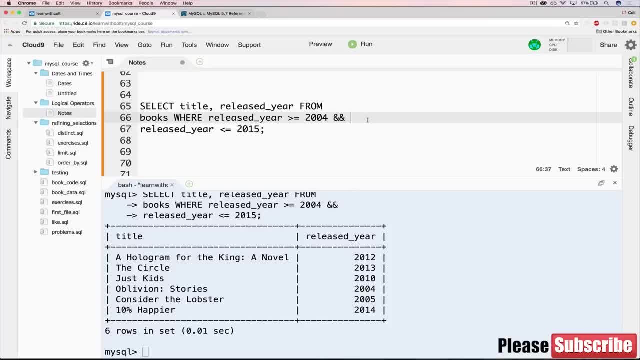 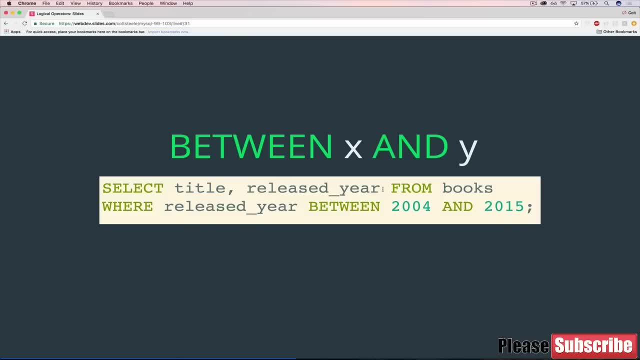 this and and this one, but they are different. So this and is paired with between always. So here's an example: Select title and release year again from books where released year between 2004 and 2015.. So this does the. 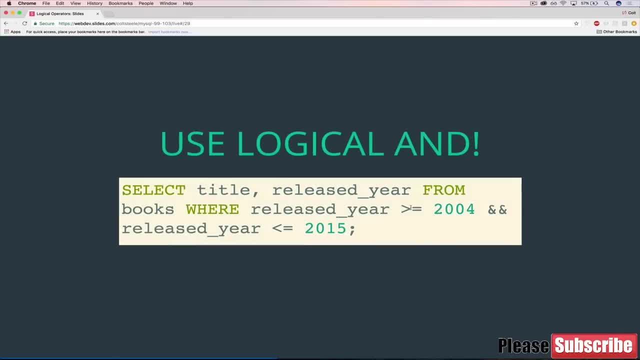 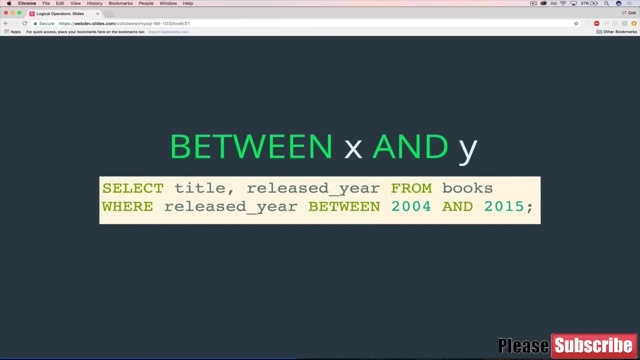 exact same thing as this right here, but we don't have to use the greater than equal to less than equal to. we don't have to write release year twice. All we have to do is say where released year between 2004 and. 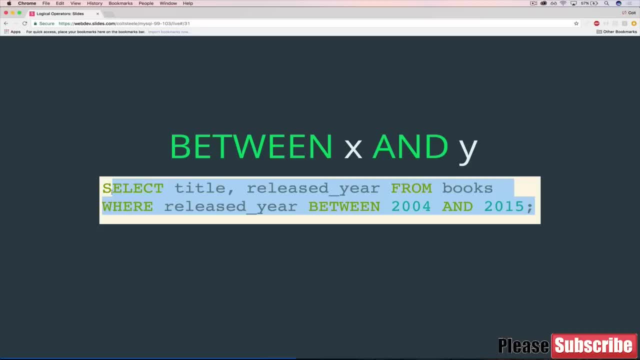 2015.. And, in my opinion, this is much easier to read, much easier to remember. if you're trying to do this, Between is a pretty straight forward thing to recall. it does what it sounds like, So let's try it out. 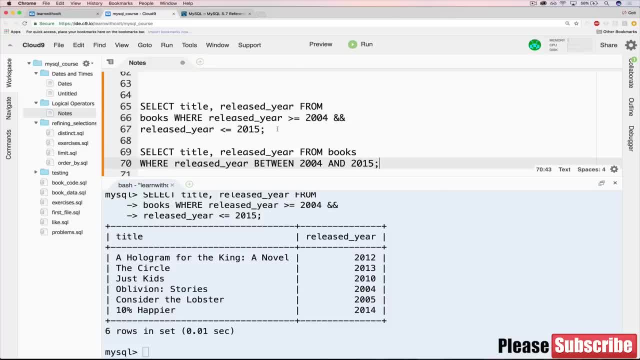 Just copy it, I'll bring it here so we have a record in the notes, And then I'll just paste it in Select title: release year from books where released year between 2004 and 2015.. And, as you can see, 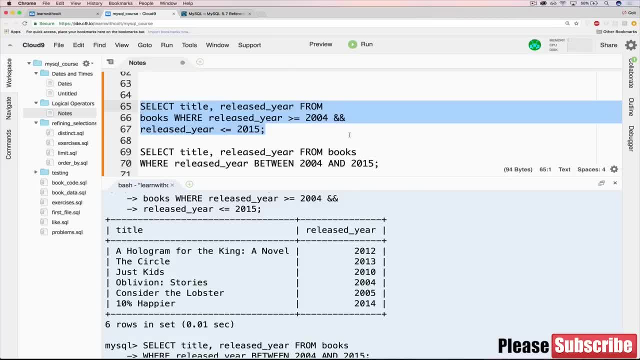 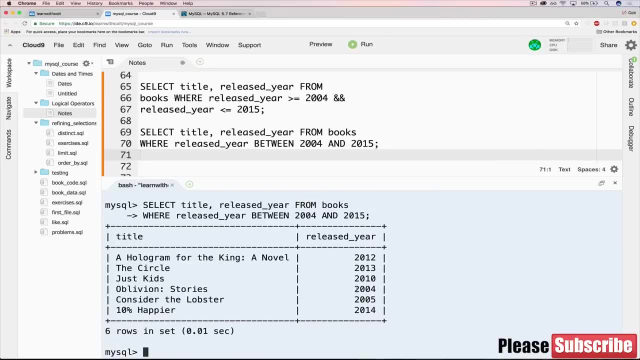 we get the same results that we did when we used this version. It's just a little shorter and cleaner and easier to understand, in my opinion, And again, it is inclusive. We have 2004 there, And one thing to keep in mind is that there may be times where you 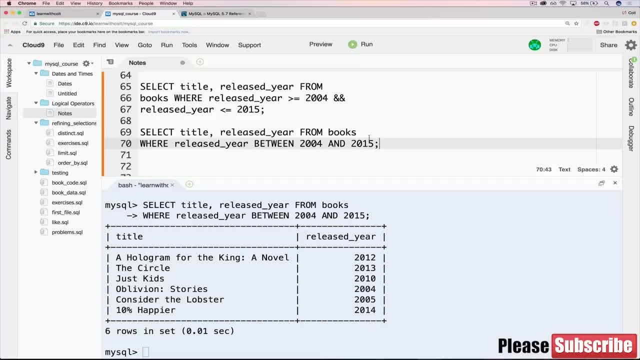 don't want it to be inclusive And there's not an easy way just to do that. Well, there is an easy way, but it basically just means change this number. If you want it to be between 2005 to 2014, you could do that. 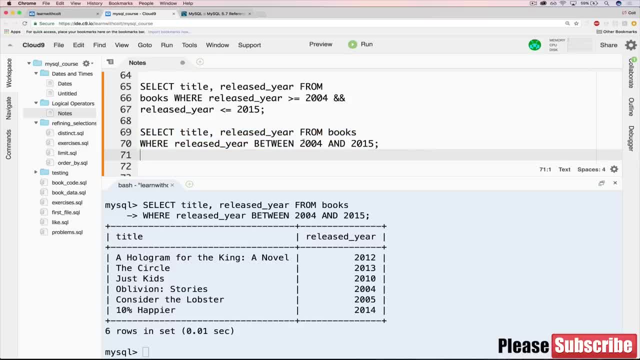 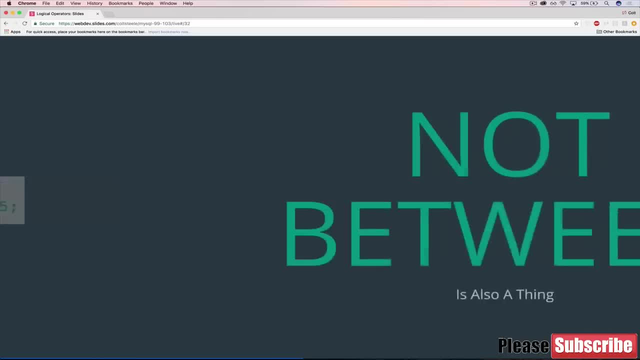 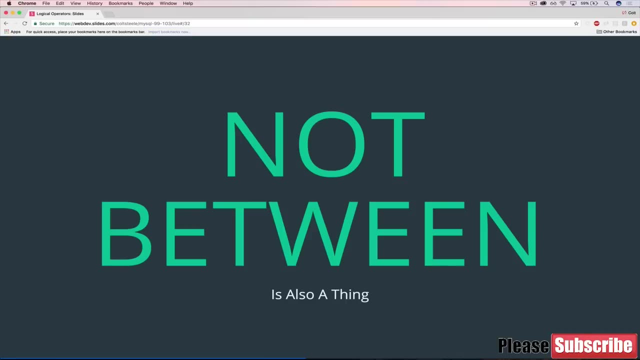 But there's no easy way to do between non-inclusive like here, where we can just eliminate the equal sign, Okay. So one other thing is that not between is also a thing, And it's pretty straight forward. Basically, it does the opposite of between. 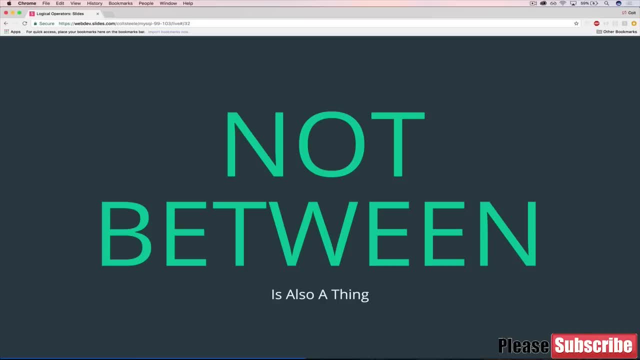 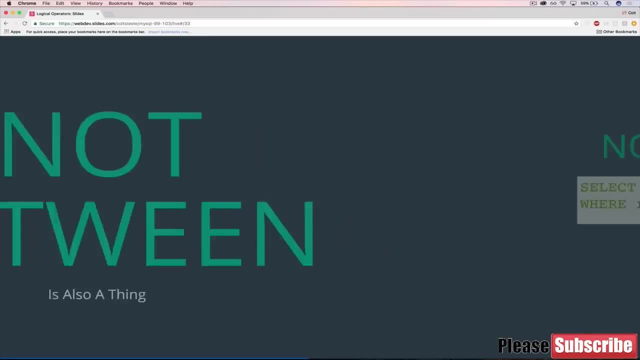 So we could say: I want all the books that have a page length that is not between 500. And that gives us everything less than 100 and everything greater than 500.. So here's our same example. If we do select title and release year from books, where 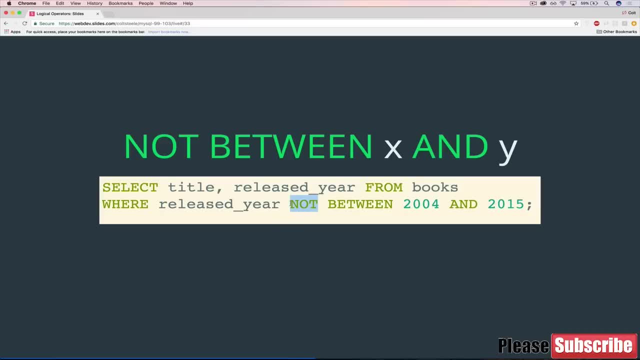 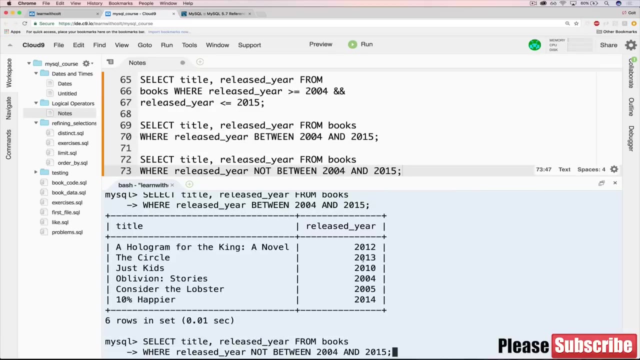 release year is not between. so all that changes is we add an OT before, not between, 2004 and 2015. it takes that range from 2004 and 2015 and does everything outside of that, So I'll just paste it here and then paste it in again. 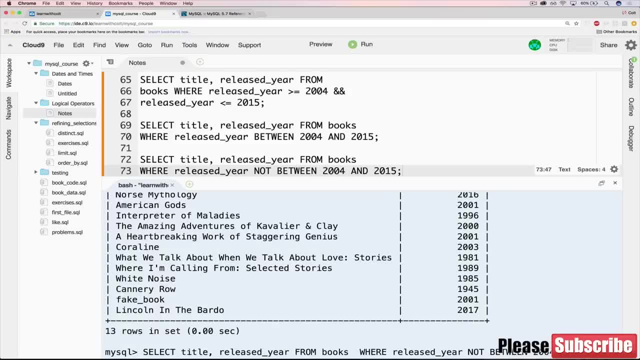 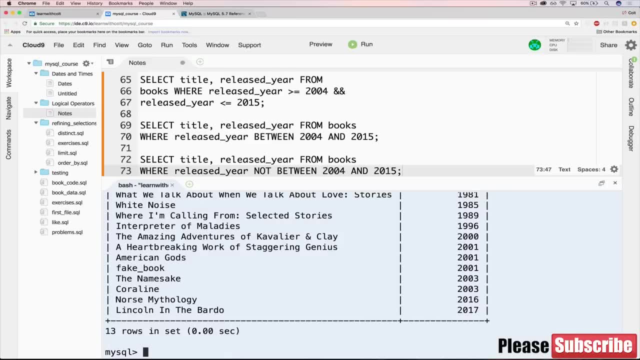 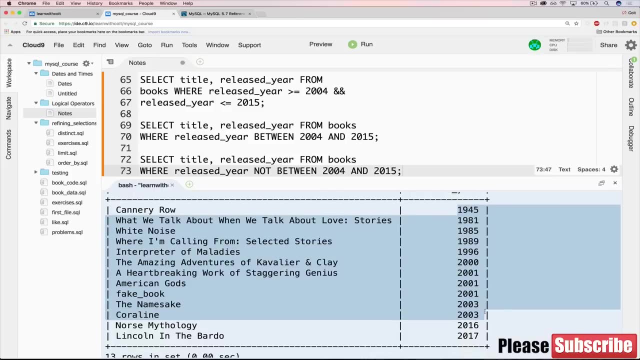 And now you can see- let's do an order. by Now you can see we have everything up until 2004 and then everything after 2015, but nothing from 2004 up to 2015.. They're gone. These are just the leftovers. 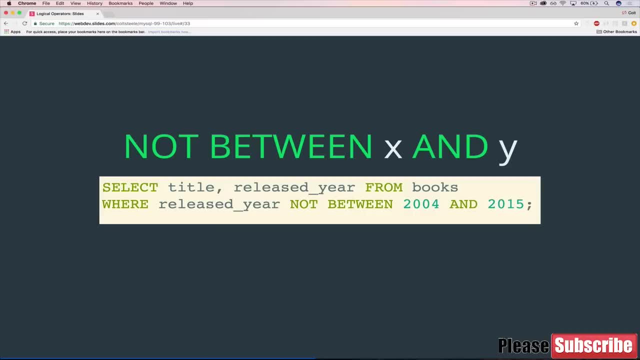 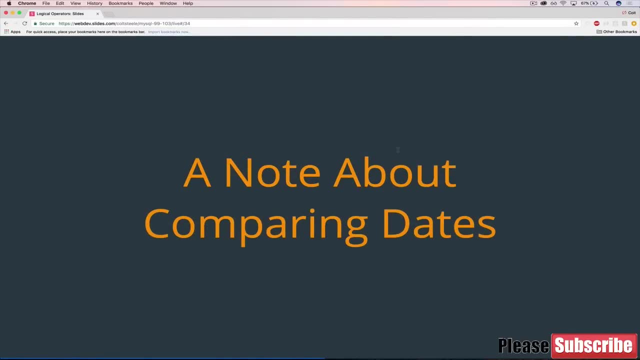 Okay, So that's pretty much it for the basics of between and not between. So before I let you go, there's one small side note I just want to bring up. It's not crucial to understanding between, but it's just something that the documentation mentions. so I figured 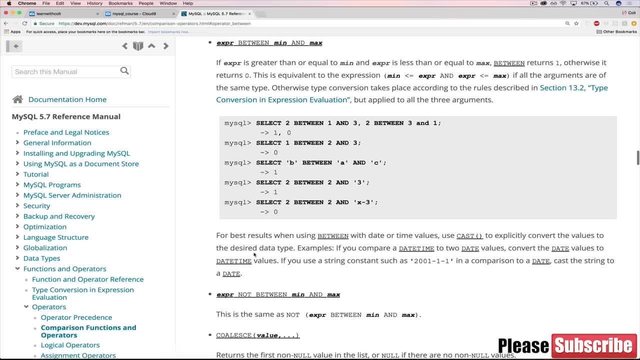 I should also mention it. If we go to the docs for between, there's this note at the end: For best results when using between with date or time values, use cast to explicitly convert the values to the desired data type. So we haven't seen this. 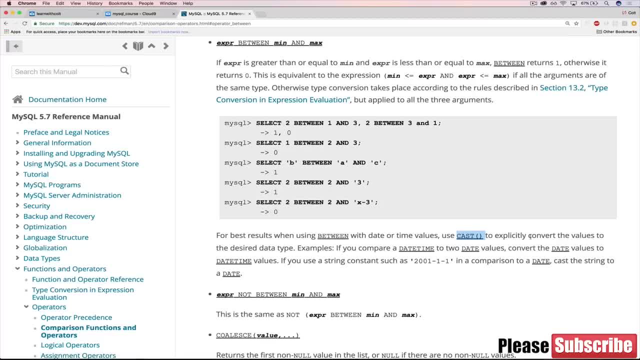 cast. I'll talk about it in a moment. But what it lets us do is convert from one data type to another, From a date to a date time, for instance, Or from a string of rchar to a date, For example, if you compare date time to two date. 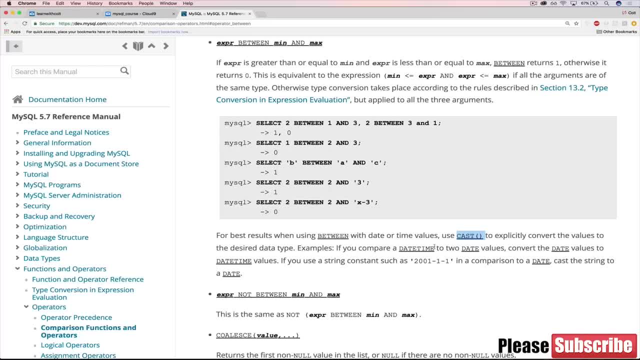 values. So we're trying to say if some date time is between two different dates, it's best to convert the date values to also be date times, Just so that you're working with the same kind of consistent data type. If you use a string constant, such as 2001-1-1. 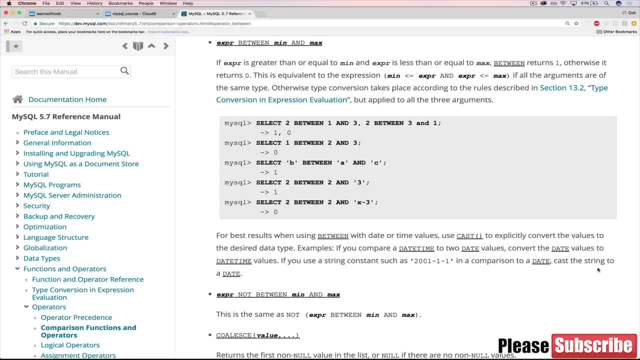 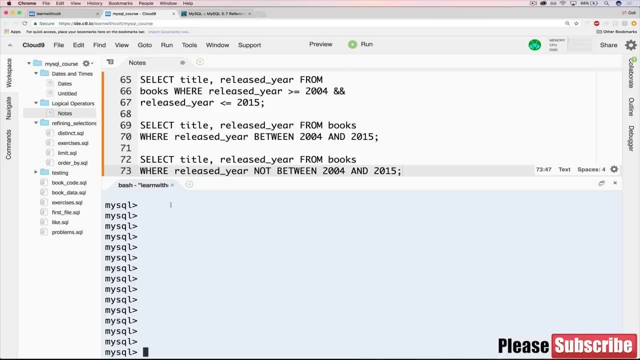 and you compare it to a date. It's better to cast the string to a date. So let's just take a look at how cast works first, And it's pretty simple. So let's take something like this: 2017-05-02. 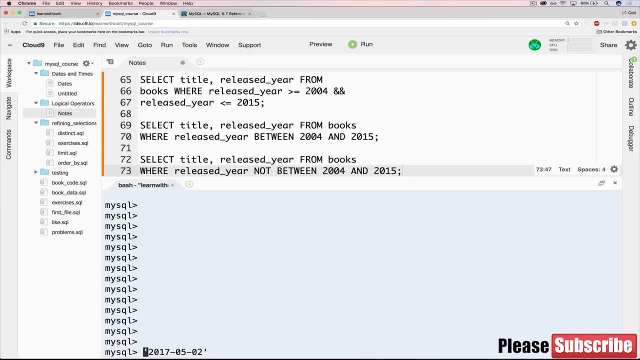 That right. there is not technically a date right. That's not considered a date data type, It's just text, Even though it looks like a date and it can be treated like one. MySQL is smart enough to figure that out if we pass. 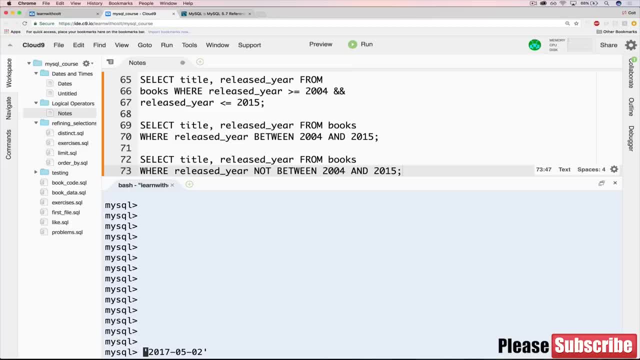 it into a date function like days or months or format date, But it's not actually a date. But if we wanted to make it an actual date time, we can cast it And this will work its magic. Now, just casting it like this won't do anything. I have to say what to? 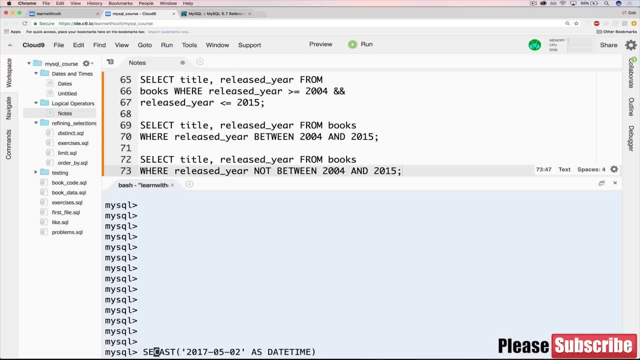 cast it as: So let's cast it as a date time And we won't see anything unless we have select here. So what this will do is it takes the first thing, whatever it is, and it tries to convert it to a date time. So if there's just 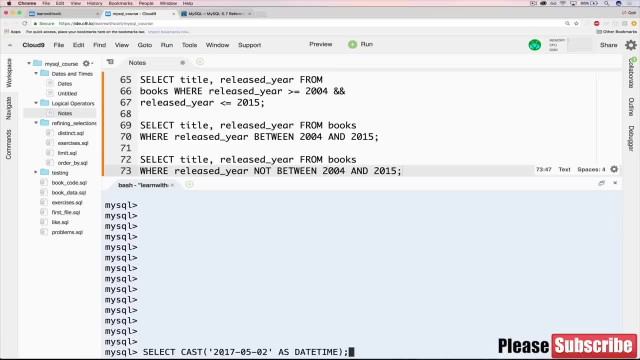 the number 99 or something that will cause a problem. But in this case this is easily castable to a date time. But you might be wondering: okay, the date part is easy to cast, What about the time part? Well, it just picks 0000 for you. 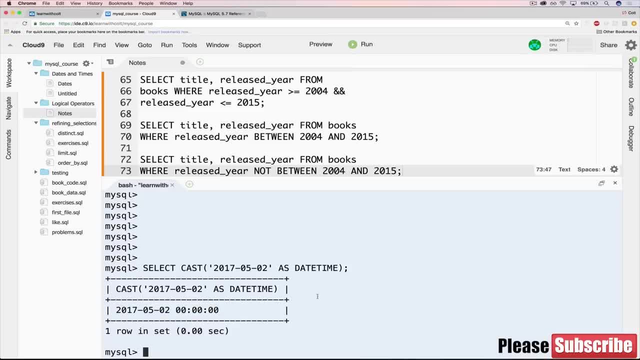 So it's now considered a date time. So basically, what the documentation is saying is, if you're working with dates and you're trying to compare them and you're working with between, for example, it's best to use cast to make sure that all the data types are the same. 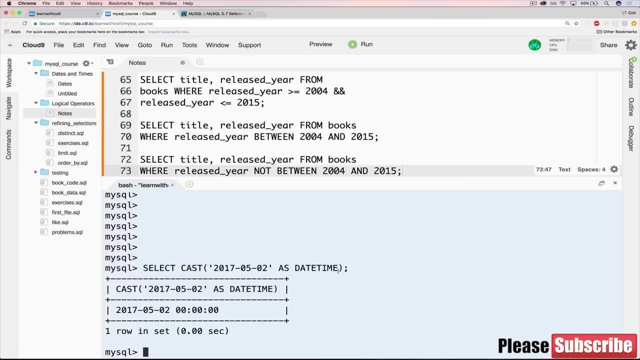 Now it actually. this is kind of confusing. it will work most of the time, just fine if you don't, because MySQL is smart enough to figure out what you want, But it can cause problems, So it's just best to do that. So I'm going to. 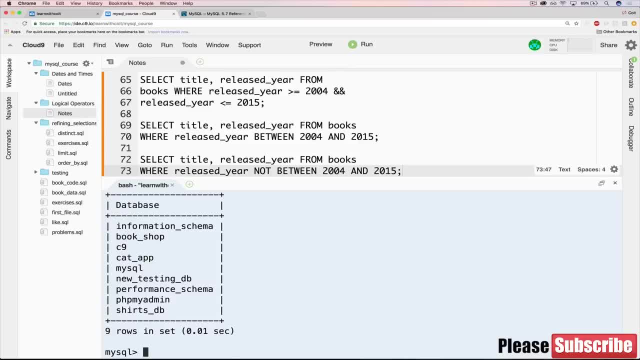 switch over to that testing database I made with this wonderful name, use testing DB. And the only reason I'm doing this is so that we have some date data. So we have a people table and they have a birth date, birth time and birth date. 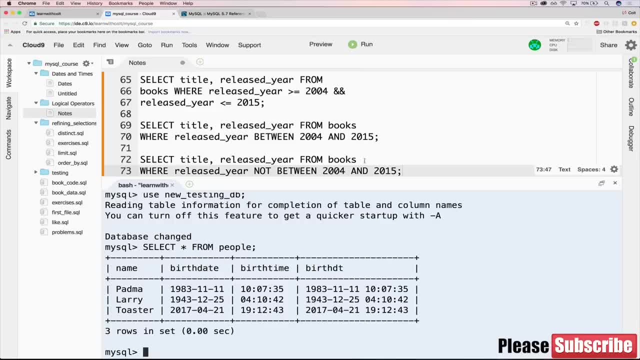 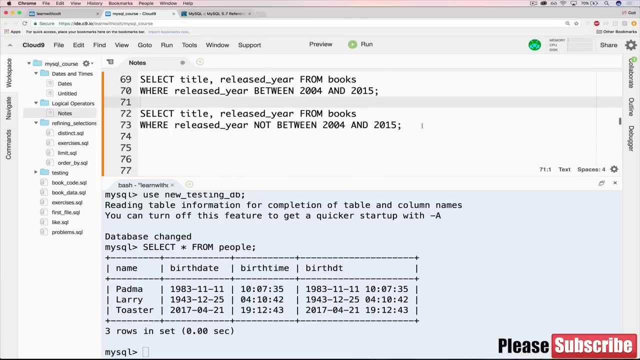 time. So let's say I want to select people who have a birth date time between two dates, Let's say between 1980, let's do January 1st 1980 and January 1st 2000.. So I'm going to write it up here. 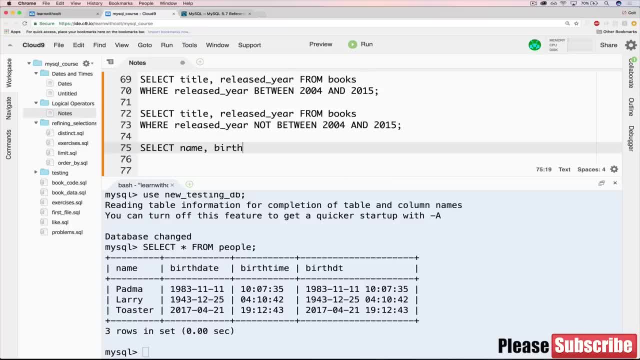 but the basics would be: select name and we'll do birth date time from people where birth date time between and if we just do this, 2000 or what I say, 1980- dash 01- dash 01 and 2000 dash 0101. 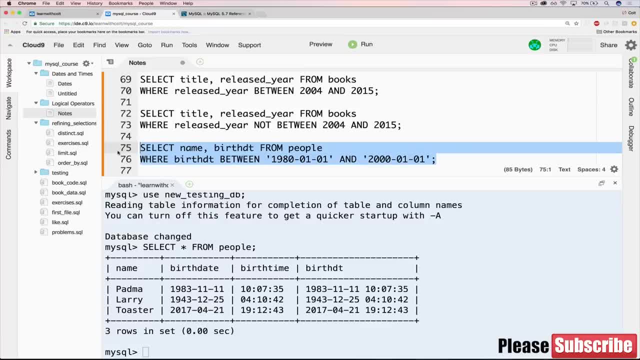 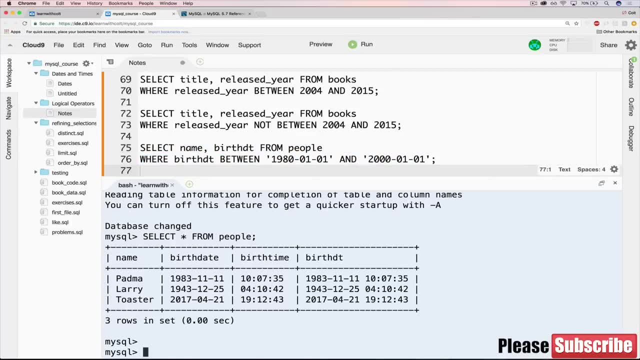 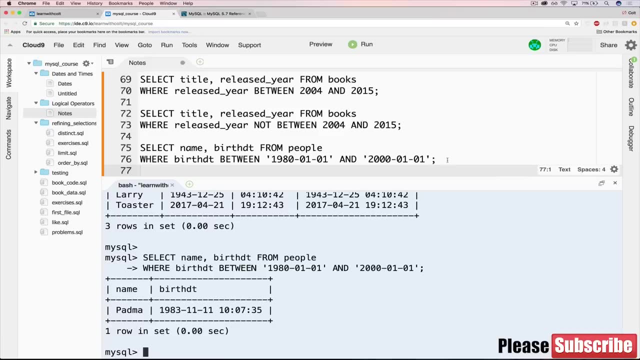 if I just do this on its own. first thing that we're doing here is: these are strings, right, these aren't even dates. technically it's text, but if I do this, it still works, and that's what I was mentioning. that's kind of weird is that it works fine enough because MySQL. 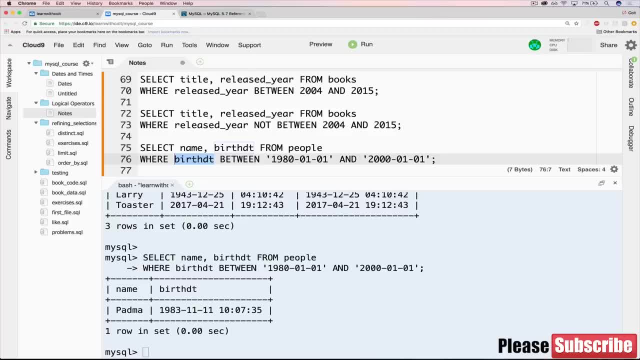 is smart enough, it figures out. okay, this is a date time. we're trying to compare it, see if it's between these two things. what are these? well, they're not date times, but we still can handle it. there's some contingency code written back in MySQL to make that. 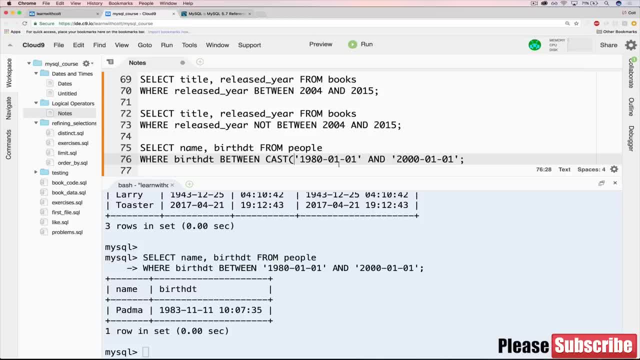 work, but it's much smarter and more fail proof to do this, cast this as date time, and I'll do this second part on a new line and cast this as a date time as well, so that we're working with date time, date time, date time, and you won't see a difference here. 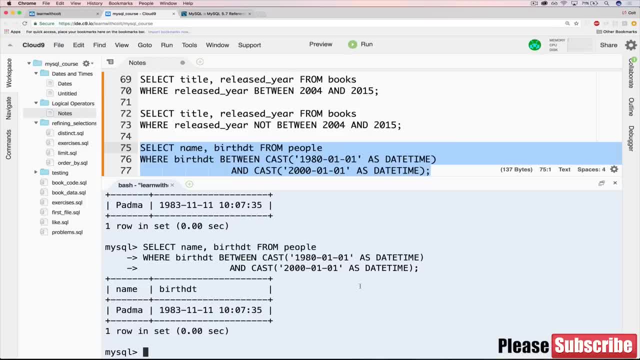 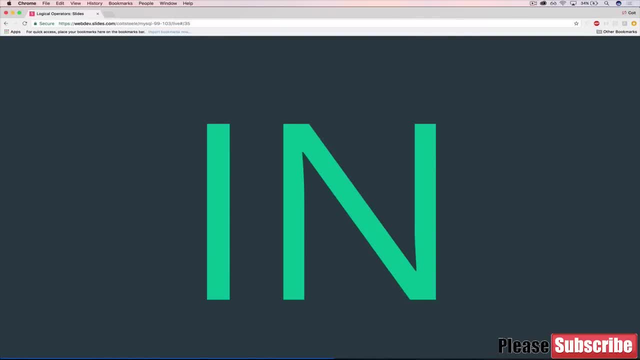 but you can rest easier, you can sleep better at night, knowing that you're doing the right thing. okay, we're done, alrighty. so next up, we're talking about a new operator called in, and what it does is it allows us to provide a set of values: 2, 3. 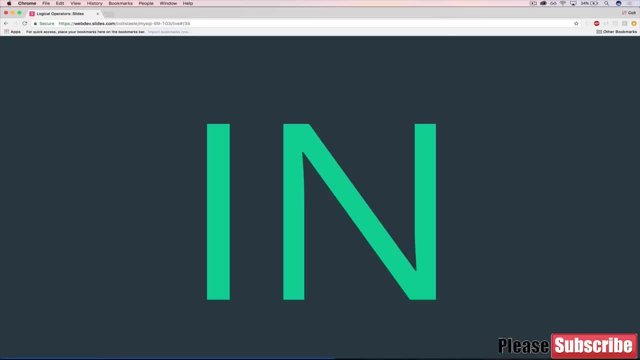 10, 50 different values and then check if a given column is in that set. so basically- let me put that in an easier to understand way- say we wanted to do this. I want to select all the books written by Carver, Raymond Carver or Lahiri. 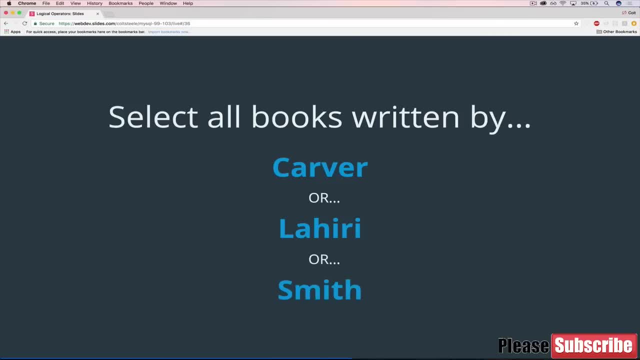 or Smith, in our case Patty Smith. so we know how to do that right now. I mean, if you listen to how I just said that with these or's you would say: select all books written by Carver or by Lahiri or by Smith, it would look. 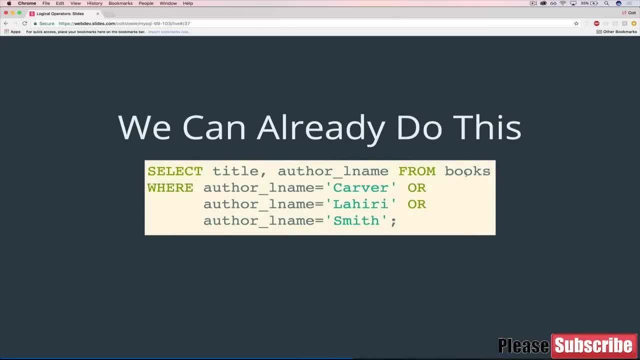 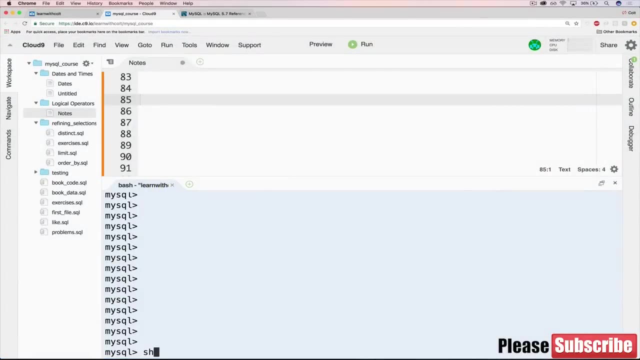 something like this: select title and author last name from books where author last name is equal to Carver, or author last name is equal to Lahiri, or author last name is equal to Smith. so this works. I'll come on over to cloud 9. first thing I'll need to do is 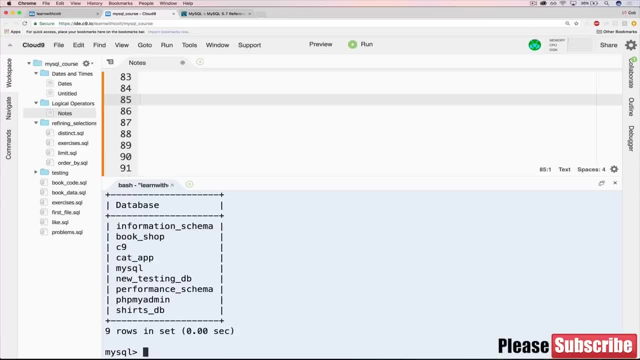 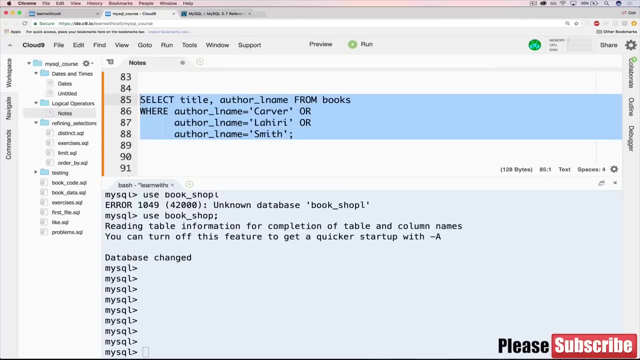 switch databases. I'm using the new testing DB, so I'm going to use book shop again. okay, so now I'm going to use this select title and author last name from these three, or from where author is one of these three. if I paste that in, you can see we get all the 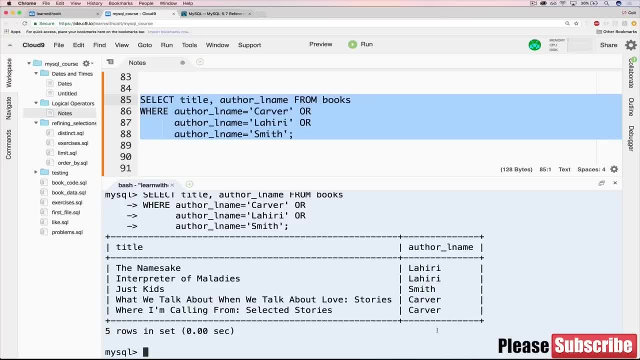 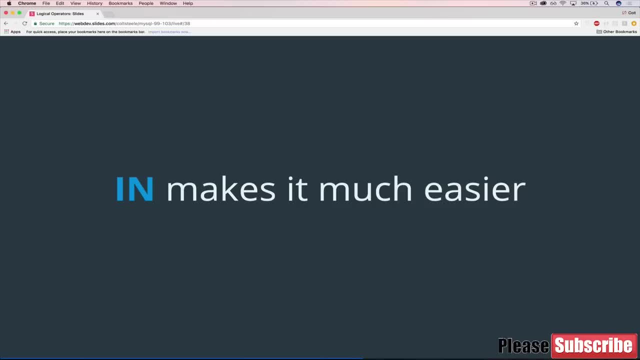 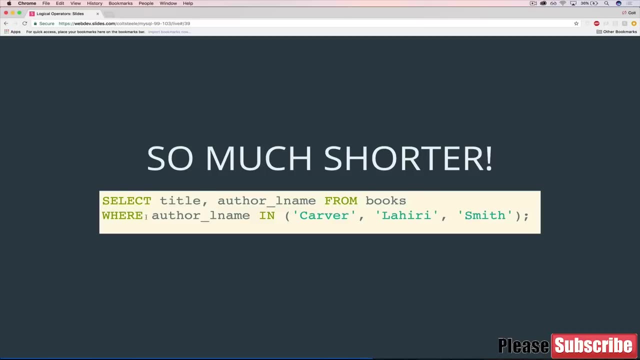 books by Lahiri, Smith and Carver perfect. however, as you probably guessed, there's a better way to do it. in will make it much easier and much shorter. so it looks like this: select title and author from the first book or from books- same thing- where author last name is. 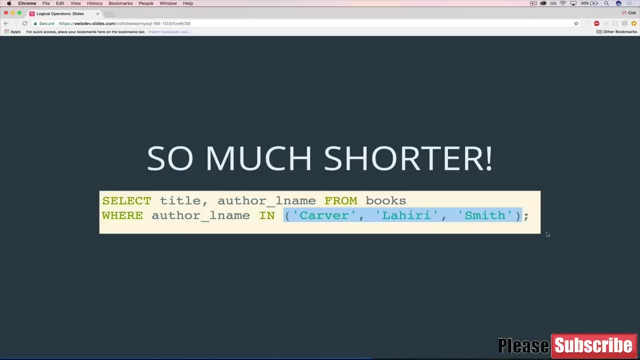 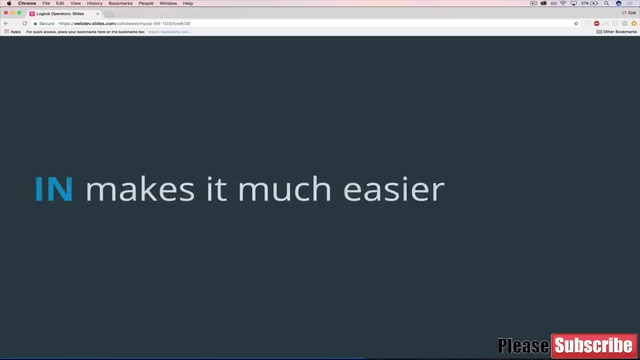 in and then in parentheses we pass in a comma separated list of values. so if author lname matches anything in here, it will be. the row will be selected. so it's really straightforward, very simple to use. basically goes from this: multiple lines and look at how much repetition. 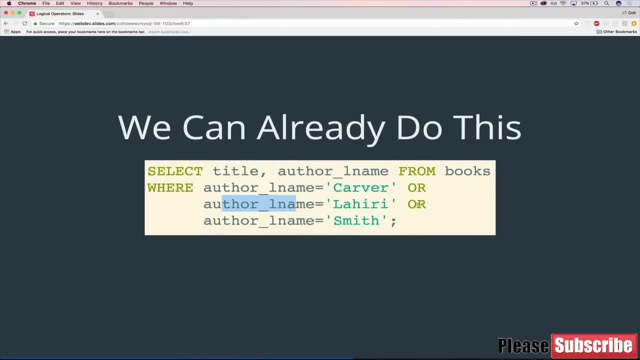 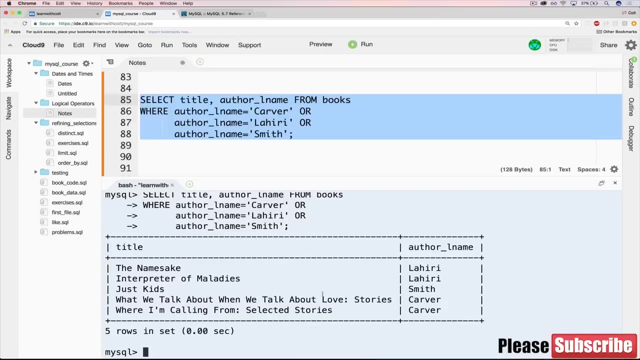 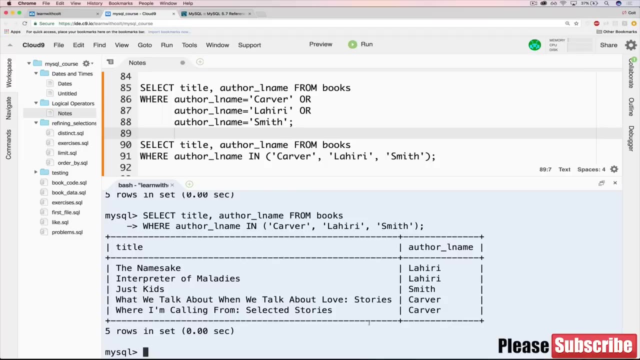 we have author lname equals or author lname equals or author lname equals and condenses it down to this. so let's try it out. I'll paste this down here so you can just compare. if we paste it in, you can see it does the exact same thing and 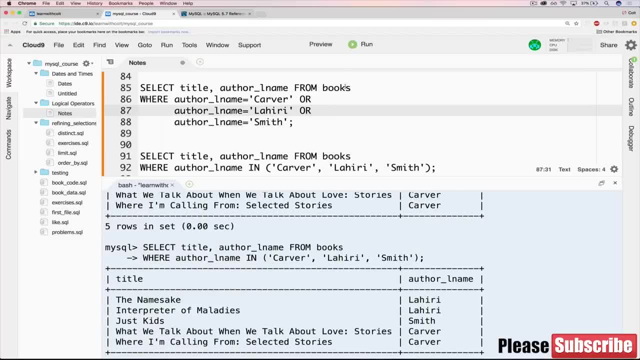 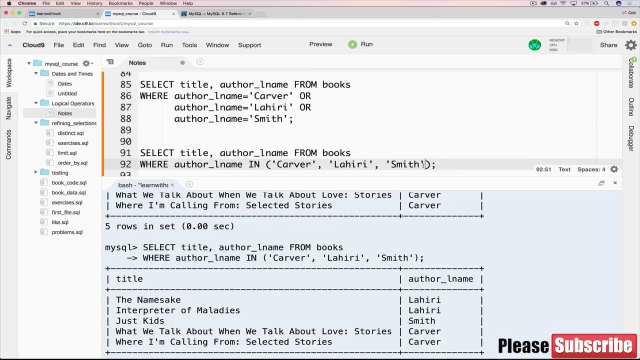 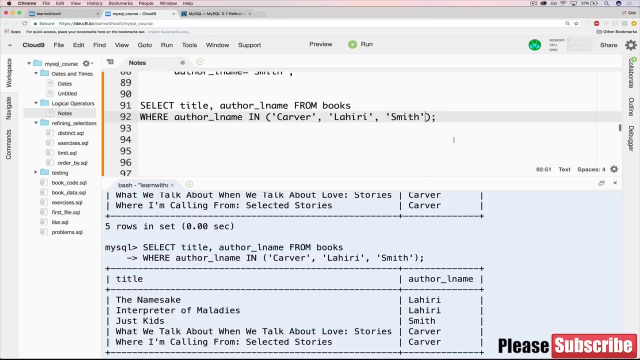 the other good thing is that you know, as we add in more conditions or more authors, in our case, this continues to get much longer every time. this is really just a very simple change. if we also want to add in another author, very easy. so it's pretty useful. 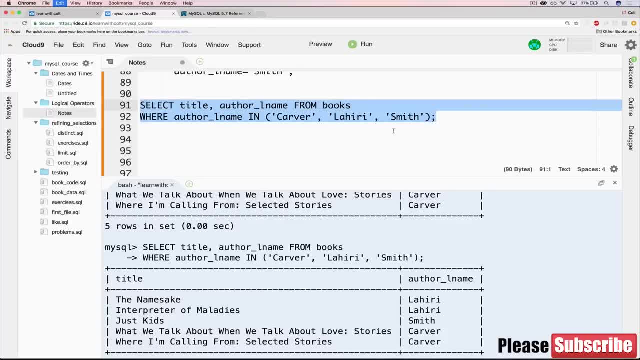 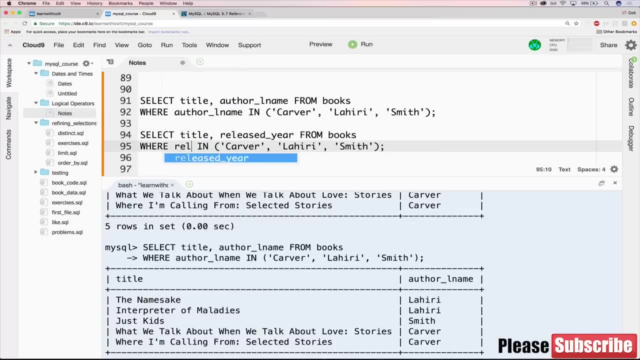 you're not limited just to working with text, so I'll just duplicate this just to show you. we could do select title and released year where released year is in, let's say 2017 or 1985, just like that. and if we paste that in, we get. 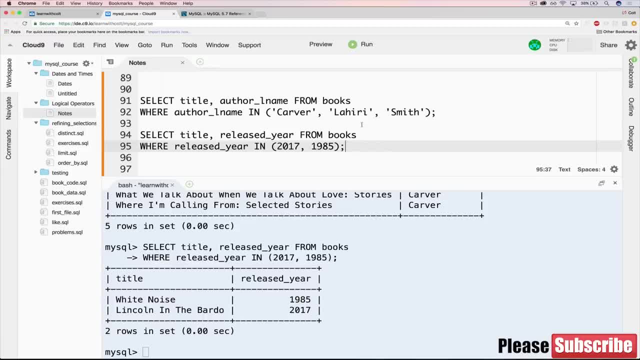 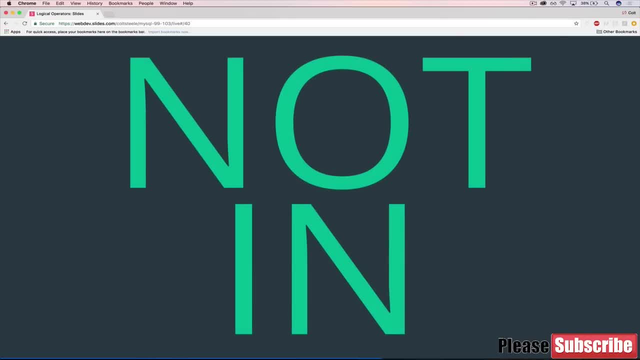 these two books. alright, so that was just to show you it doesn't have to be strings, you can work with numbers as well, as you probably guessed- maybe you didn't, I don't know- but there's also a not in and it works just like not between works compared to between. 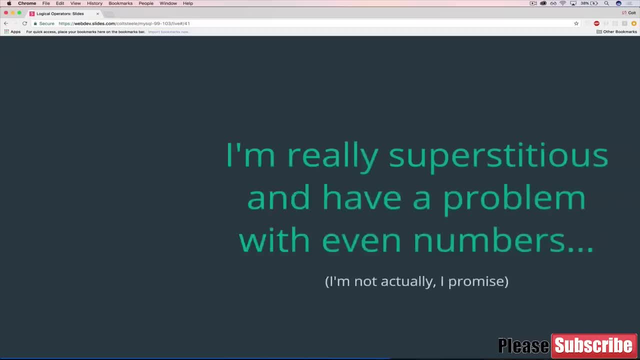 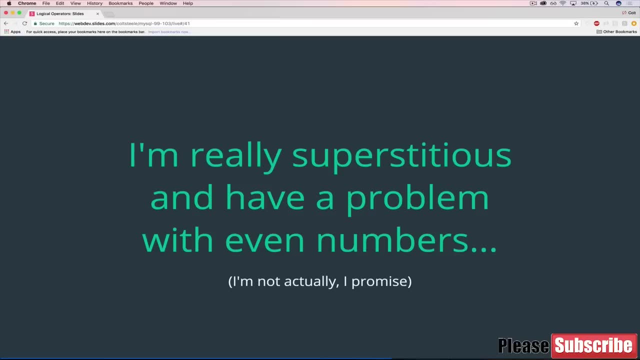 it will do the opposite of in. so let's say this is a really dumb hypothetical. but let's say I'm really superstitious and I have a problem with even numbers. I go into the book store and I tell the clerk this, even though I promise I'm not superstitious. 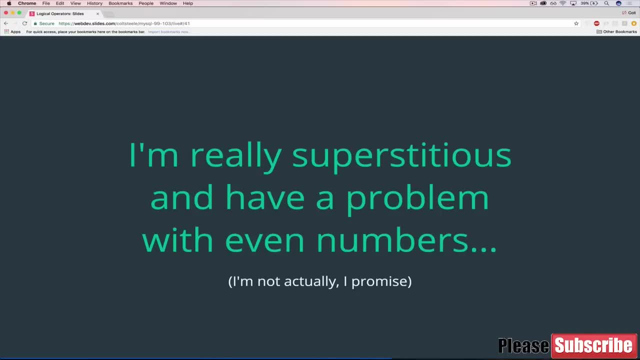 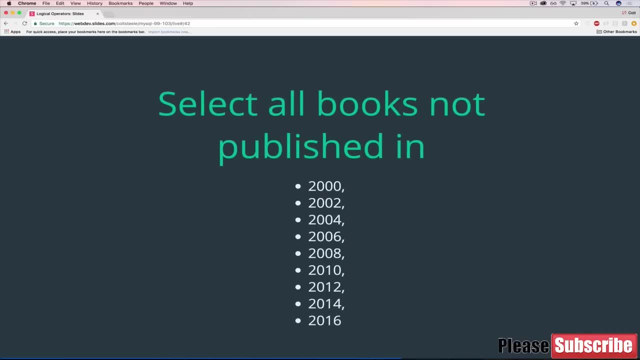 and I don't have a problem with even numbers, if anything. I really like even numbers if you can. but I go into the store and I say I want to get all books that were not published in even number- years 2000 until 2016. so I want to exclude 2000,, 2002. 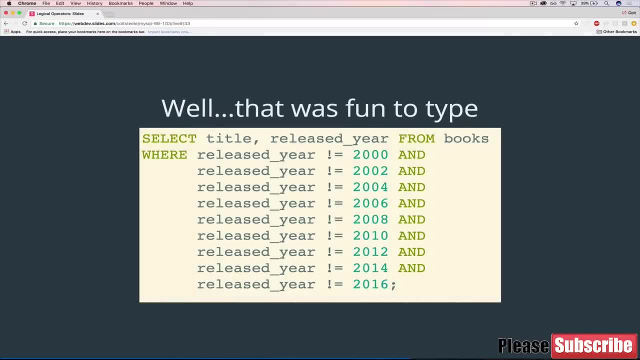 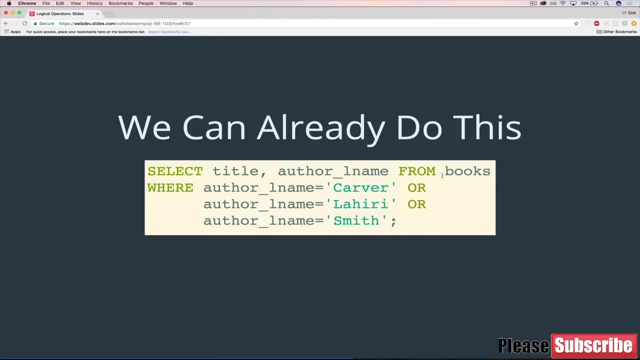 2004 and so on. well, I do this, which is kind of a nightmare, where I'm basically using logical ands and not equals. so remember- I'm going to have to go back a few slides here- when we were doing this version here before we talked about in. 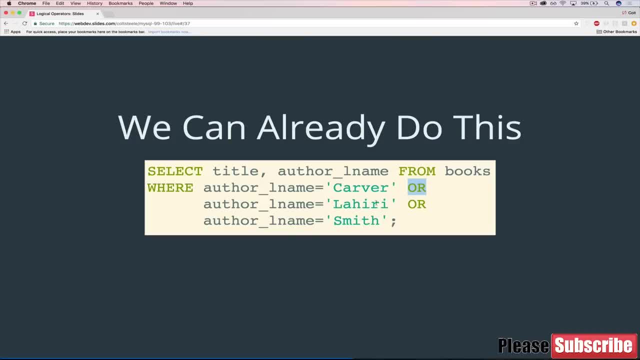 I was doing equals and or so authorlname equals carver or authorlname equals lahiri. but when we negate it- and I want to do the opposite- I need to negate the equals with a, not equals or to an and which. when I say it that way, 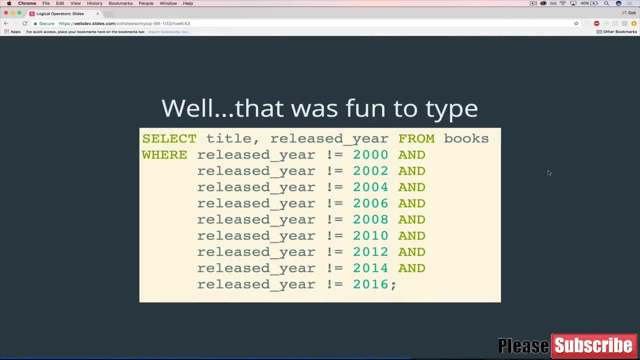 I realize it may sound a bit more intimidating than it is basically. logically, if we step through this, what I'm saying is I want to select all the books where released year is not 2000 and it's not 2002 and it's not 2004 and it's not any of these. 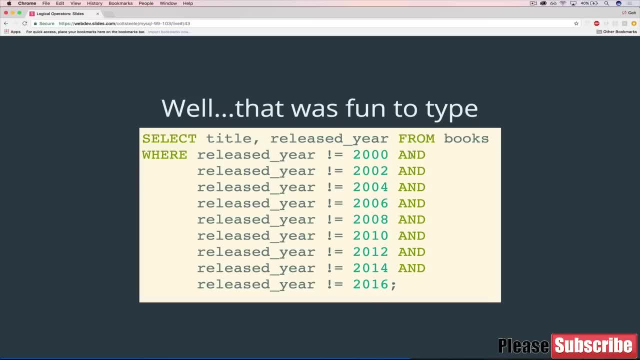 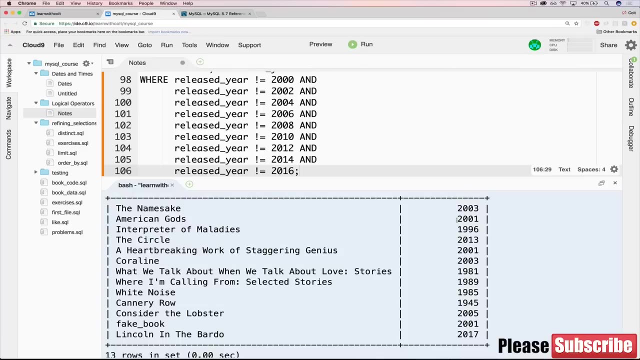 so anything other than these values and or wouldn't work here. it has to be and ok. but the point is that this is a mess. it's obnoxious, it's gigantic. if I do copy it over and I try running it, you'll see we get all books from. 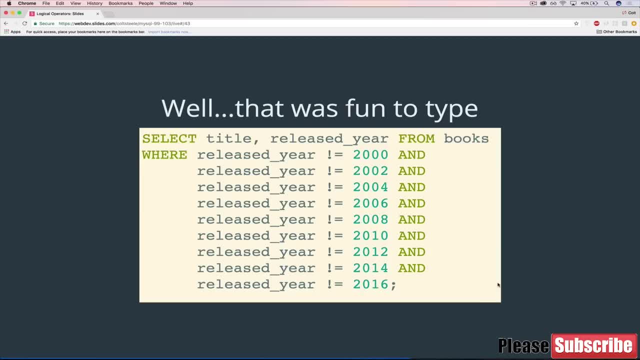 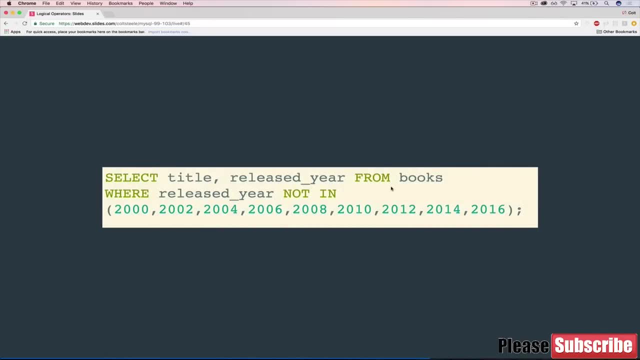 odd number years. but there's a better way we can use not in, which works just like you'd expect. rather than saying in, we just say not in and we provide that list, that set of values, and in this case I've just passed them all in. notice the difference there. 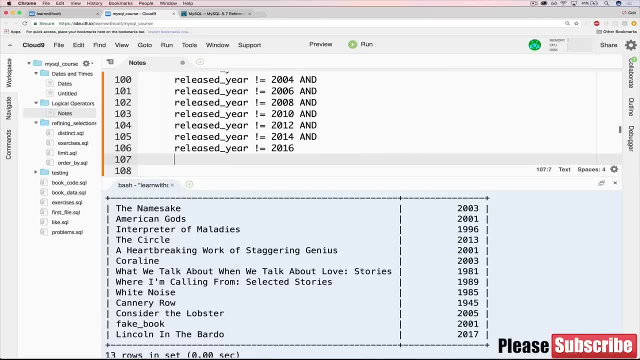 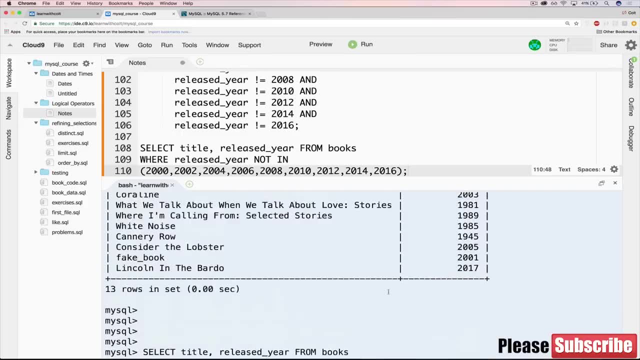 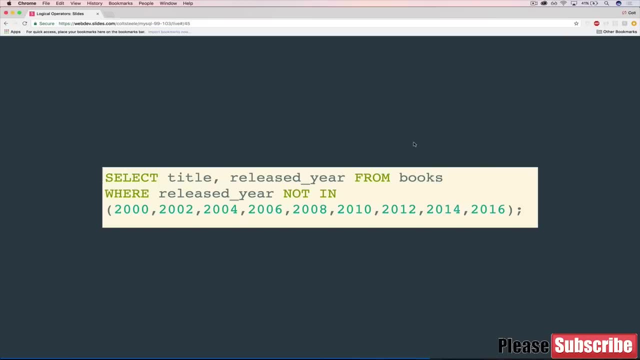 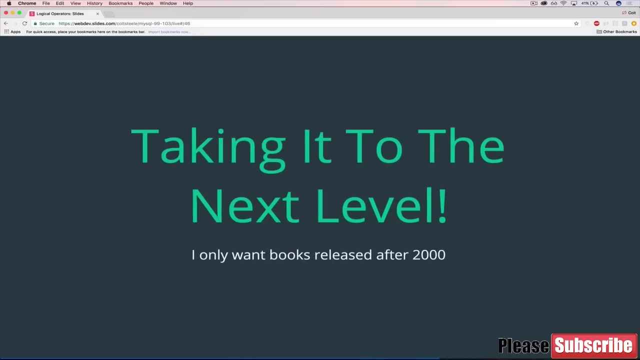 massive difference and if we run this, we get the exact same result, but much, much shorter, much easier to add onto or change. now some of you might be thinking: well, this still seems really silly. there's a couple things that we can change. one is that I only want books released after 2000. 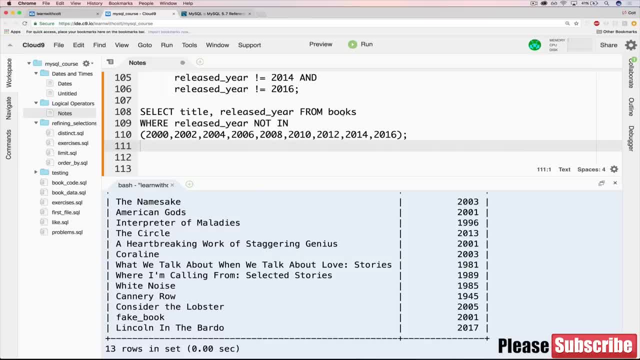 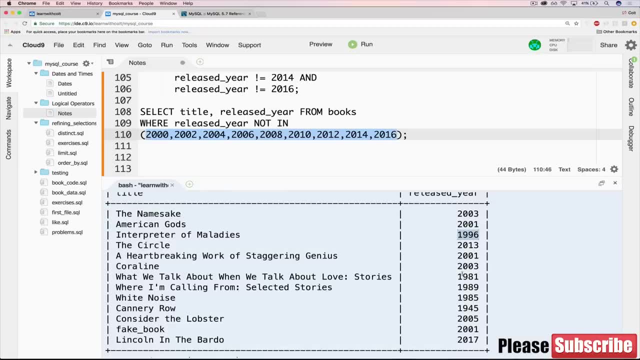 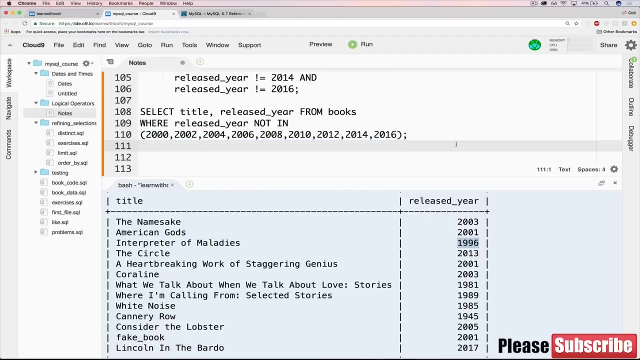 so right now I'm basically saying I don't want any, even years in the 2000s, but we're still getting even years 96. is there any others? I guess it's just 96. so what I could do is say that I only want books. 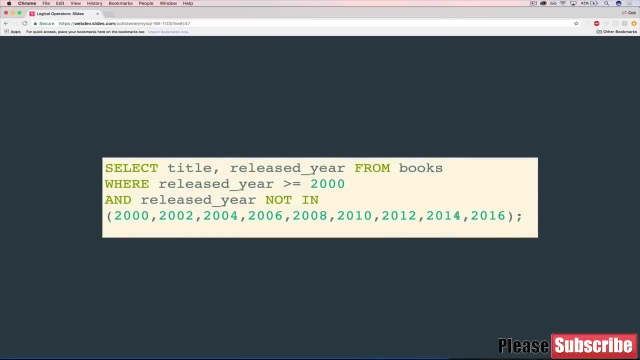 released after 2000 and it would just look like this. so the only reason I'm showing you this is so that you can see how to use logical and in conjunction with something like not in. so all that we're doing here is selecting books where they're released after the year 2000. 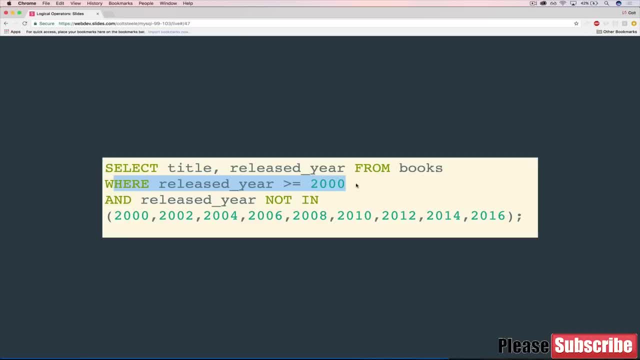 including 2000, greater than or equal to 2000. so that's going to narrow it down significantly. and then within that subset, we only want ones that were released in years that are not contained here. so the odd numbers, the odd 2000s, 2001,, 2003, and so on. 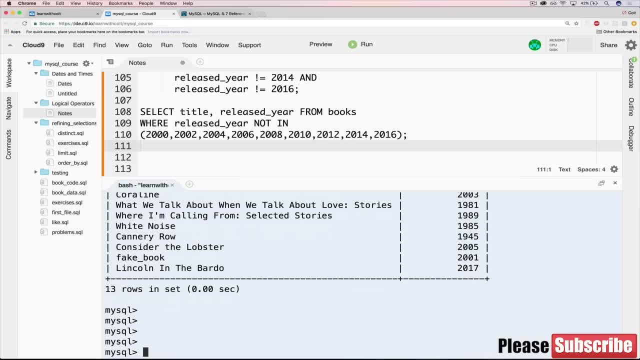 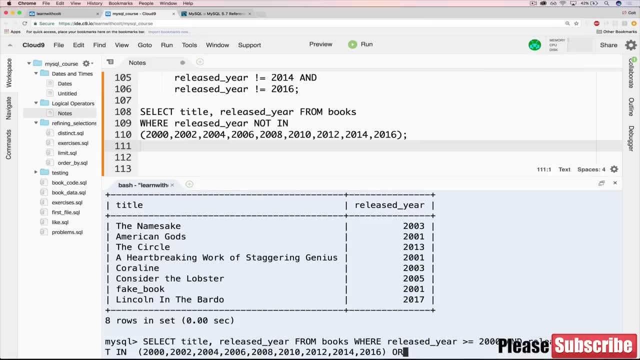 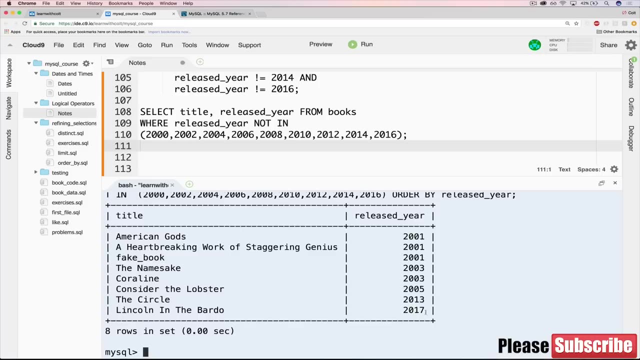 so, as far as why you would do this, let's say that I have taste in literature and I only want recent books from odd years, and let's do an order by there we go. so we get 2001 all the way up to 2017. 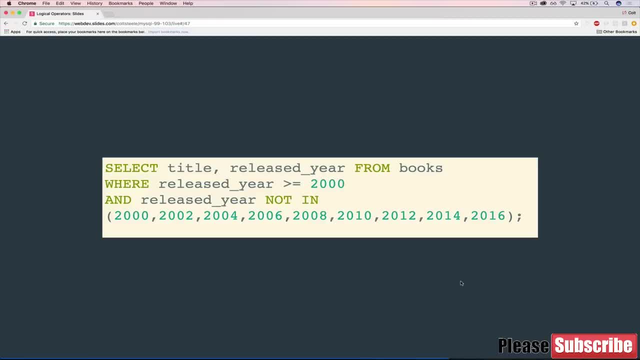 all the modern books with odd years. but there's still something more, and it doesn't require us to use in or not in, because if you look at this, this is pretty repetitive. it's long and there's a pattern here, so there has to be a better way to express this. 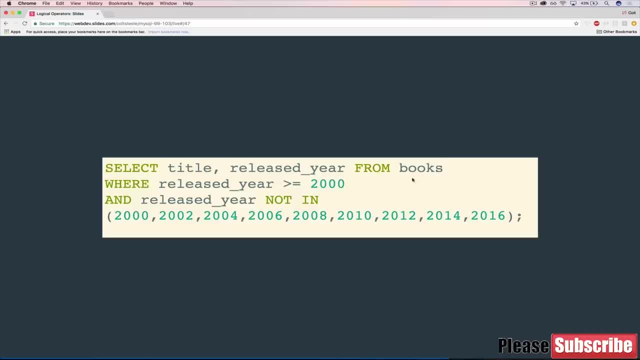 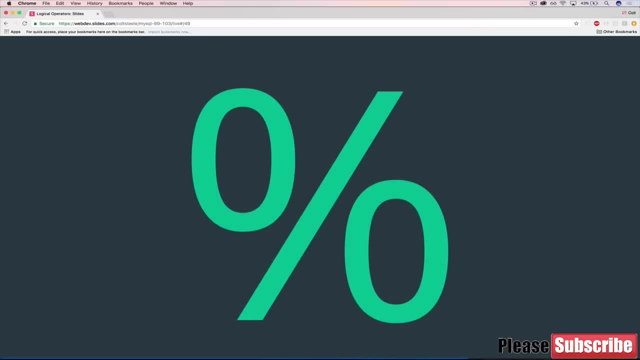 and what I'm going to show you here has nothing to do with in or not in, so it's a bit of a tangent, but I feel that it's worth talking about. if you're familiar with programming, the solution here is to use an operator called modulo. 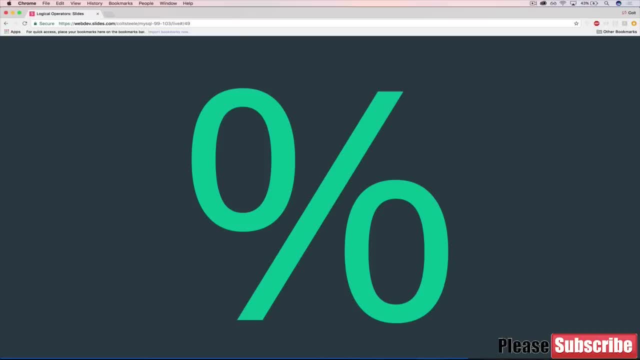 and basically, this is also known as the remainder operator. what it will allow us to do is test if something is even so. how do we know if something is even in general? well, it's divisible evenly by two if we can divide two into a number and there's no remainder. 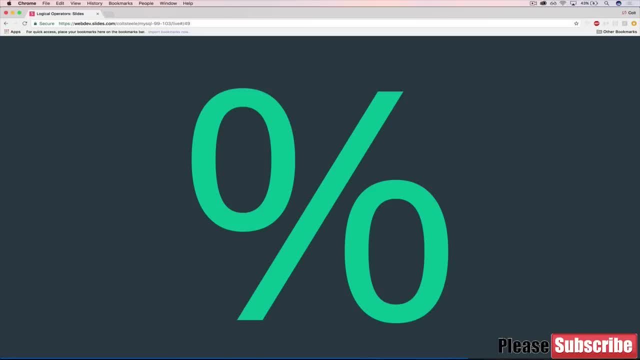 that means that it's even. two is two and it's just a whole number, so it's perfect. but three, or let's say seven, divided by two, is not a clean even division, so that means that it's not an even number. so there's a way to do that. 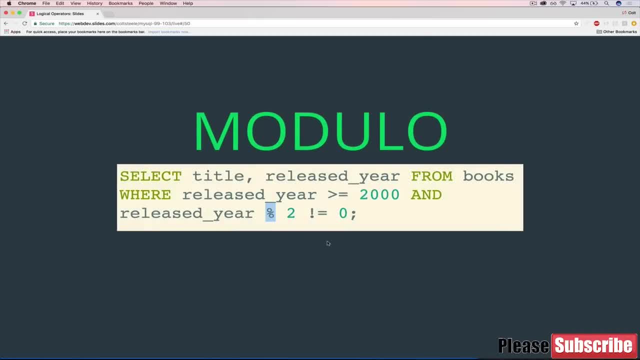 it looks like this. so the percent sign is known, as I said, as modulo, the remainder operator. so if we just focus on that part, this is saying release year divided by two, the remainder is not equal to zero. so if we plug in 2000, right here, 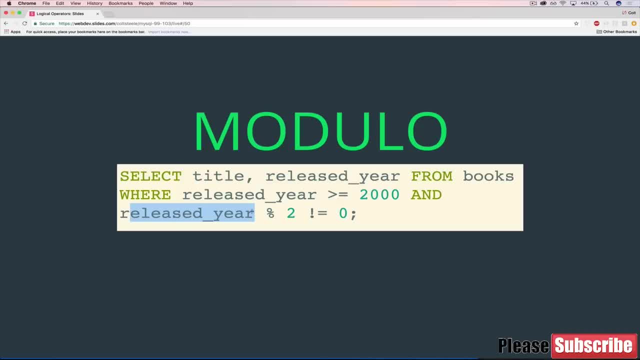 2000 divided by two, the remainder of that is zero. but if we plug in 2001, the remainder is not zero. the remainder is one, meaning that it's odd. so again, this is above and beyond what you need to know, but I just figured it would come up in the comments. 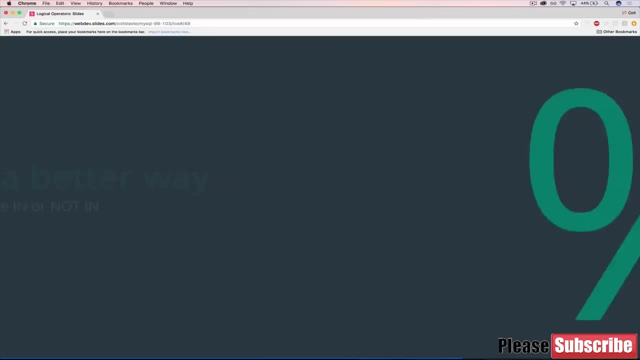 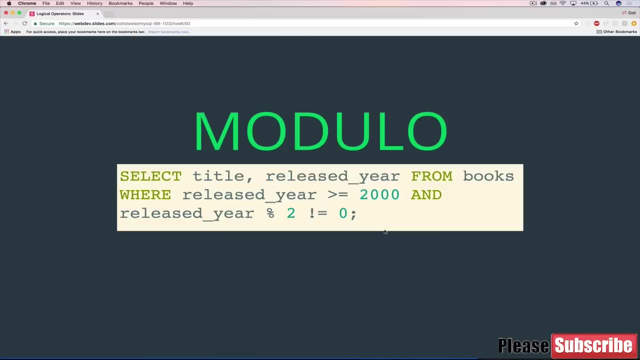 if someone saw this gigantic mess here, someone would probably say there's a better way, and they're right. it just happens to not use in, or not in the whole point of this video, but I figured it was still worth talking about. so what we're doing? selecting the same stuff. 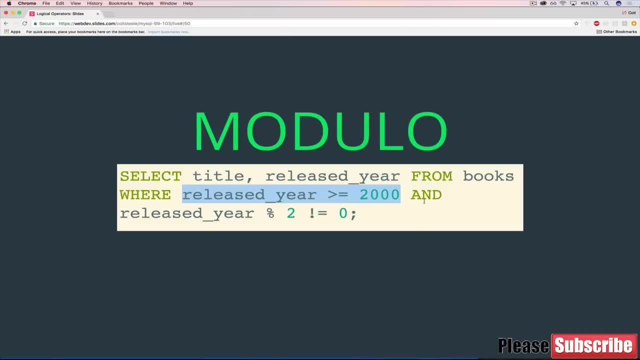 title: release year from books. first thing is the same: only selecting books that are released after the year 2000 or including the year 2000, and then they also have to be odd years. so release year is not release year. mod two is not equal to zero. 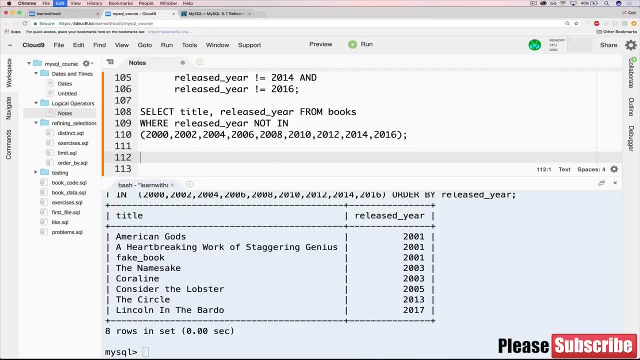 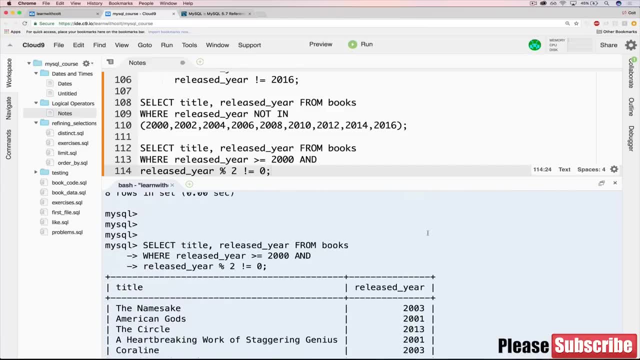 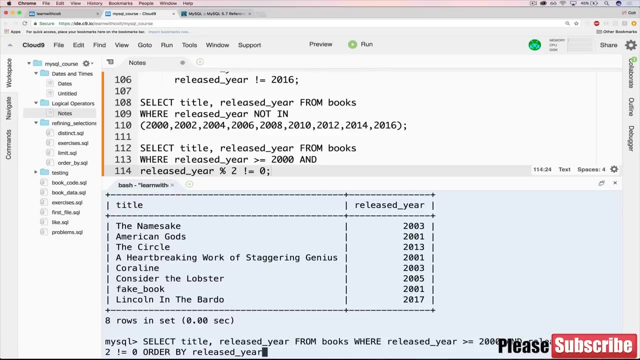 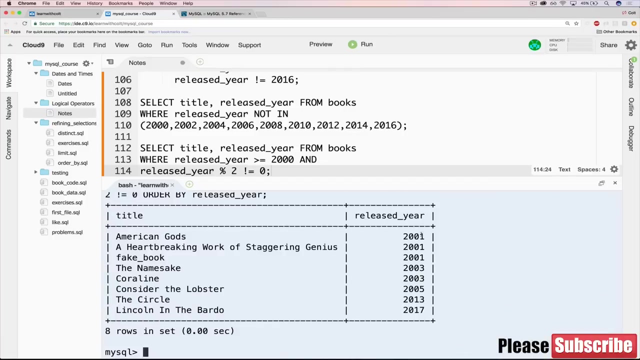 two does not divide cleanly and paste that in, just so we have a record. run it. you can see. now I only get same exact result. let me order it so that we can compare. no, I have a typo. ok, so we get the exact same results that we got earlier. 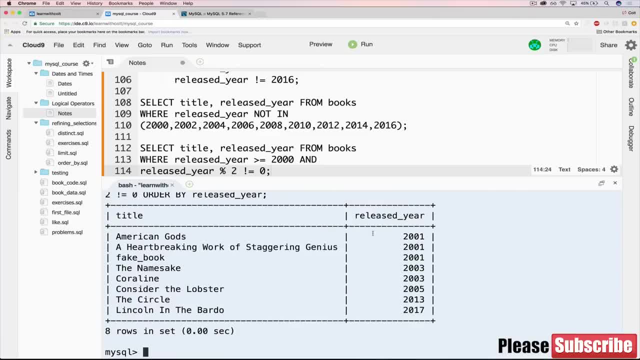 but we didn't have to write all these years out explicitly, and the other advantage is this solution works when we're in 2018 and 2020 and whatever other even numbers we have. as long as they are even and greater than 2000, it will be filtered out. 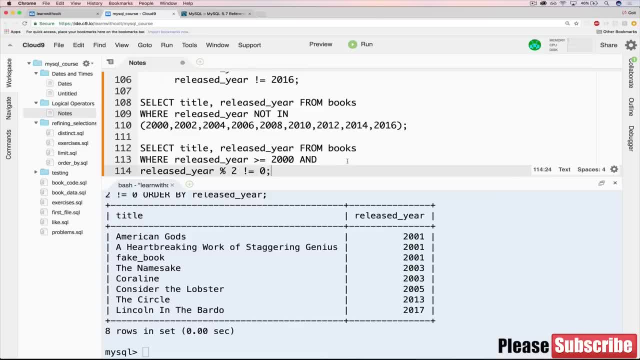 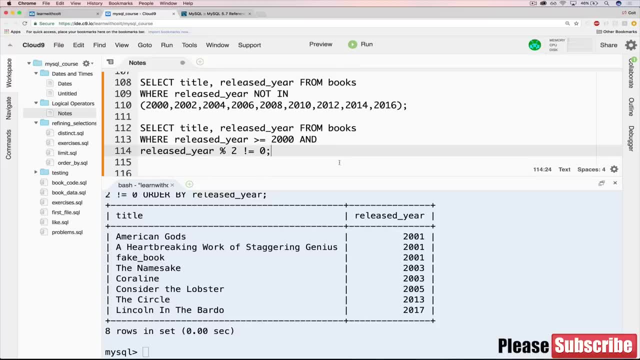 so this is, in my opinion, a better solution. it grows and it expands more. the other thing: there's a bit of a performance difference. it's not major, but when we look at this, basically, if we're pretending, let's personify or anthropomorphize MySQL. 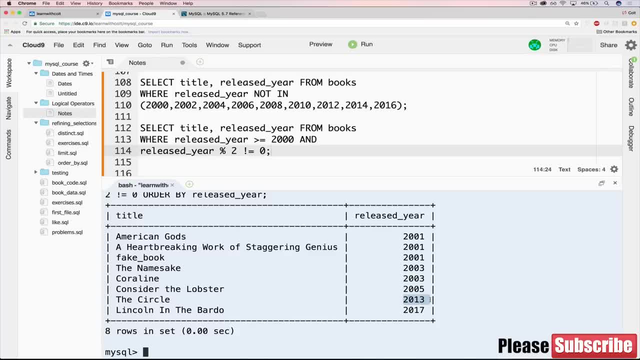 and it's taking a year, like 2013, when we have not in, it's going to try. is 2013 equal to 2000? no, is it equal to 2002. no, is it equal to 2004, and it's going to keep going down. 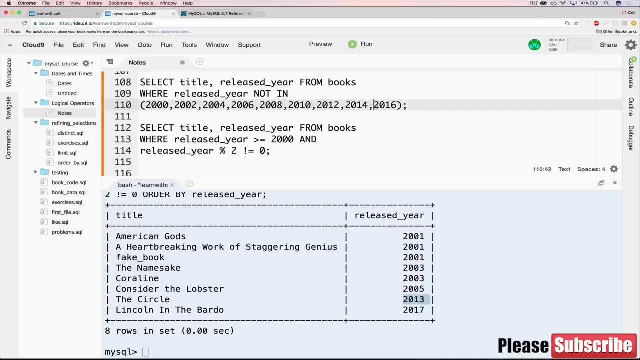 it has to try every option. there's no way to know unless it actually matches it or tries to match it against every year we have in this set. so that could potentially take a lot more time than doing a single mathematical operation like we have here. we're just checking is the release year? 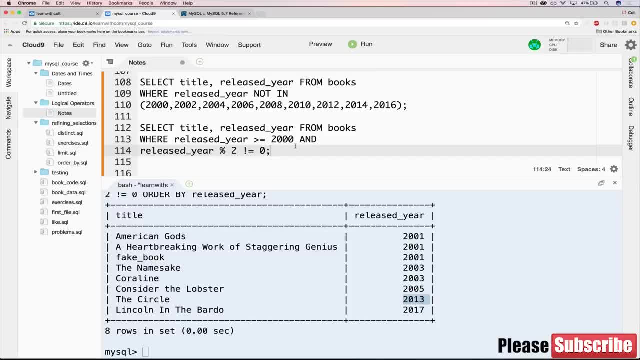 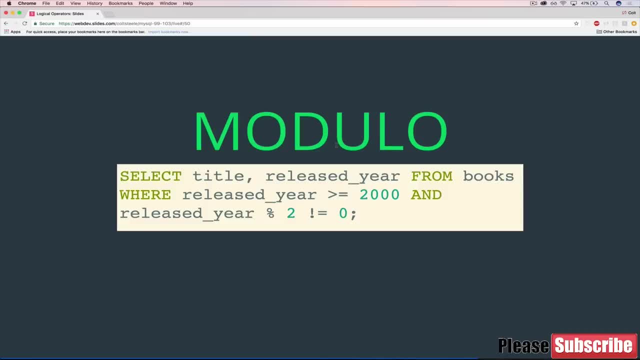 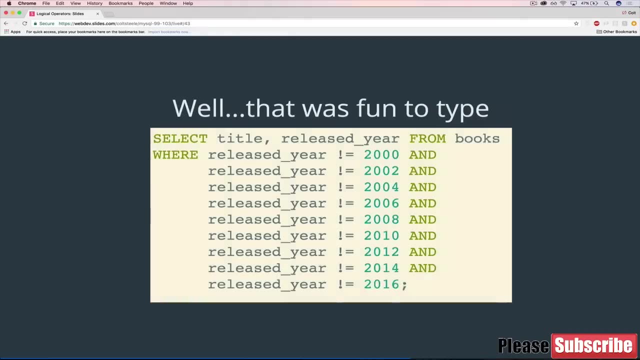 mod 2 not equal to 0, and it's really not a big difference, but it's just something that's nice to be aware of. ok, so big tangent here. this video was really about in and not in, so just to go back to there, very useful. 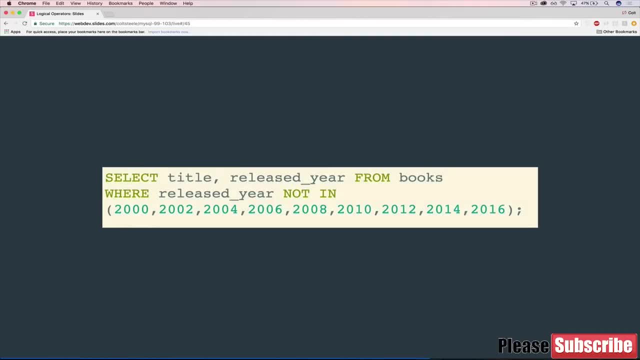 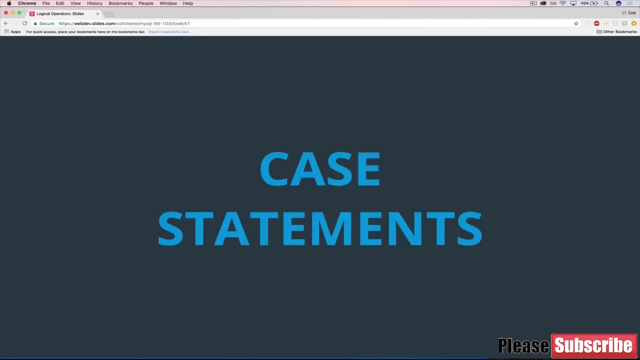 allow us to pass in a set of numbers or strings, or values, dates, whatever it is, which then our rows are checked against to see if they're either contained or not contained, depending on if we're using in or not in. ok, so we now have one more video, one new bit of. 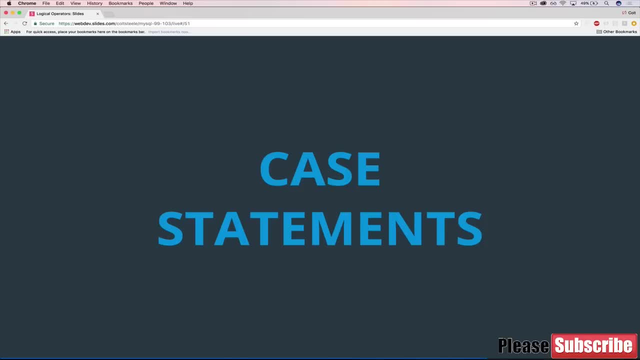 information before we move on to the exercises and wrap up this section and go on to join tables. very important, big topic. but before we do that, we have this video, which is honestly called case statements. this is a pretty well. exciting is relative. this is very different than things that we've seen in this section. 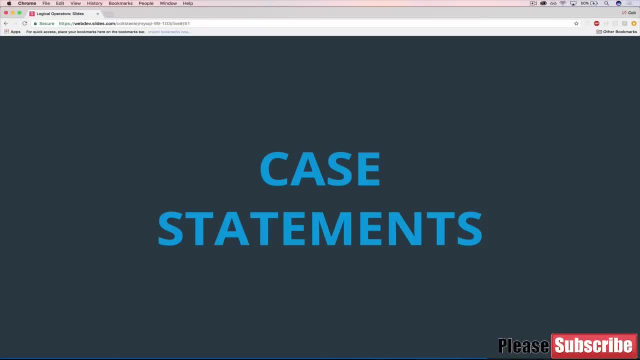 it has to do with logic, but it's kind of on a bigger scale. it allows us to make decisions. so if you're familiar with programming languages- that's something I've been saying a lot in this section- but if you are, you've probably come across case statements or conditional statements. 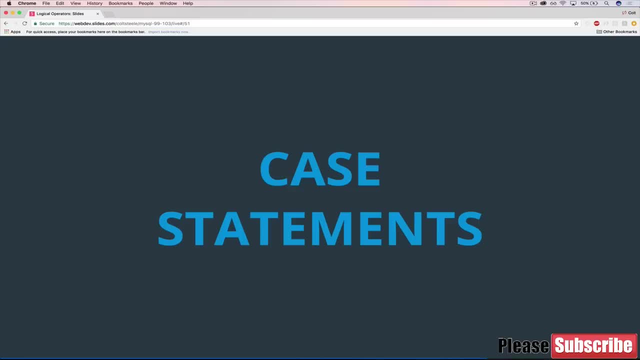 which allow you to add logic in to do things like conditionally print something out. it's a very simple example, but if a number is greater than 5, print one thing, otherwise print something else. well, the same thing holds true. in my SQL. we use these case statements. 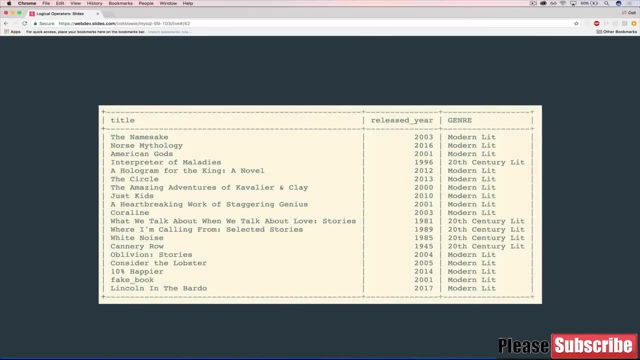 which I'll show you in just a moment- to do things like this. so over here I have a genre category or a genre column that is not in our database, and what I've gone and done is basically said, print out title and release year, which are very straight forward. 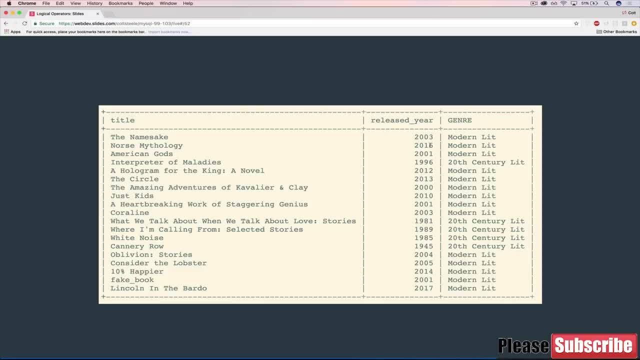 but then take that release year and if it's greater than 2000, genre should be equal to modern lit. if it's less than 2000 then it should be 20th century lit- very, very simple genres. we could easily expand that. maybe genre is the wrong word. 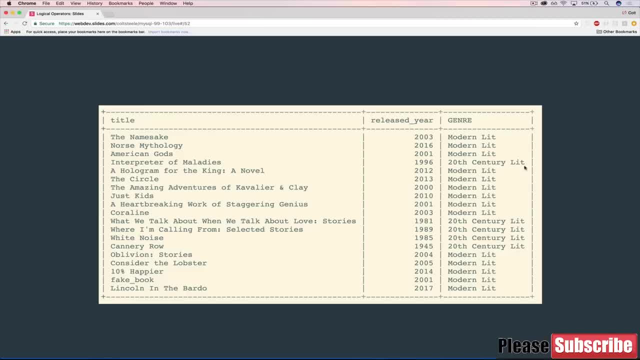 maybe period is better or era, but I called it genre. it's a lot of work to change these slides now, so we'll just call it that. but again, what's happening here is we have a conditional statement. this depends on this. so if we change release year of the namesake to be 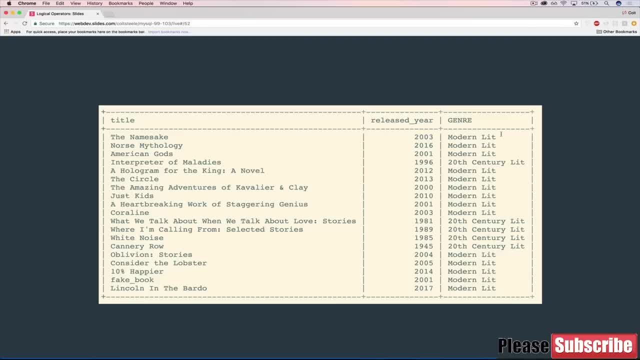 90. this would also change to be 20th century lit. so it's adding in logic a new layer of complexity that we haven't seen how to do to make these decisions, and we're not limited just to two. of course, we could break it up into. 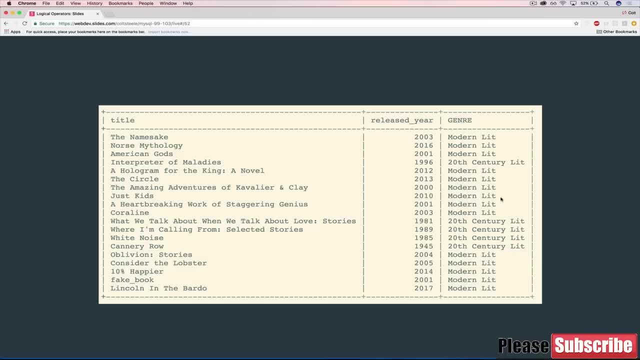 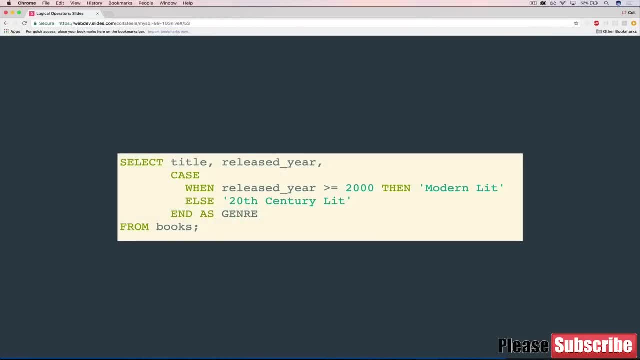 a whole bunch of things and I'll show you a few more examples. but let's first identify how this works, and I warn you, there's kind of a lot of syntax. ok, so here it is. this is what results in what we just saw. so the beginning and end are the same. 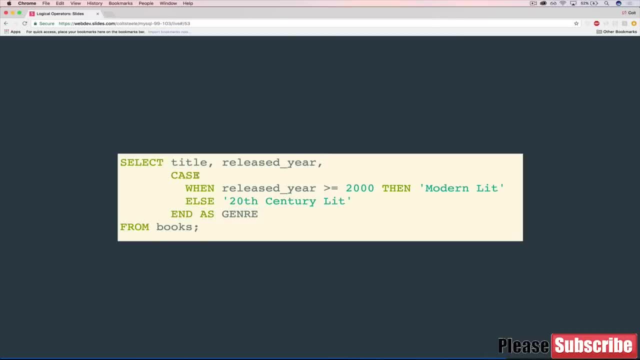 select title and release year from books, but then we have this whole case thing: four separate lines. they don't have to be separate, of course, like anything in MySQL, but it makes it a lot easier to see what's related to what. first thing that we have is: 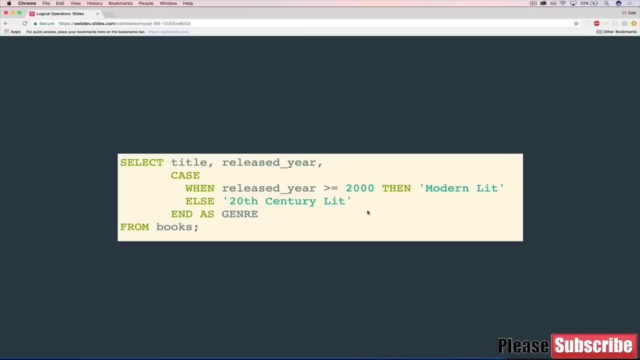 case, that's the word that says this is a case statement. it's going to consist of a couple of points of logic that will spit one thing out and that thing ends right here, and then I have an as, so I don't have to have as genre. 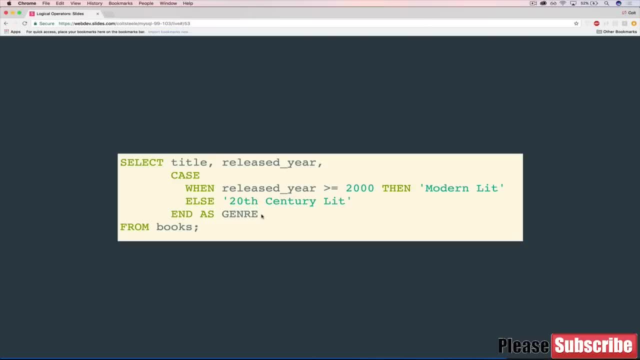 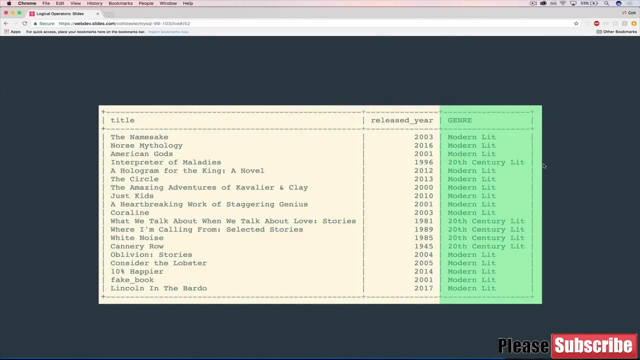 remember that's called an alias. but if I left that off it would look really, really gross when it printed out in the table, because instead of genre here it would say this entire thing, which would make the table gigantic, it would go way off the page and would ruin our formatting. 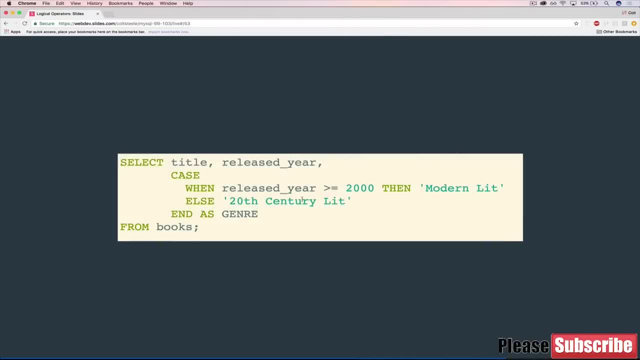 so usually want to use as. but then the more important part is what we have right here. so case statements take the following form: there's always a when, at least one, and then there's an else, as well as the opening case and the closing end. so let's step through what this says. 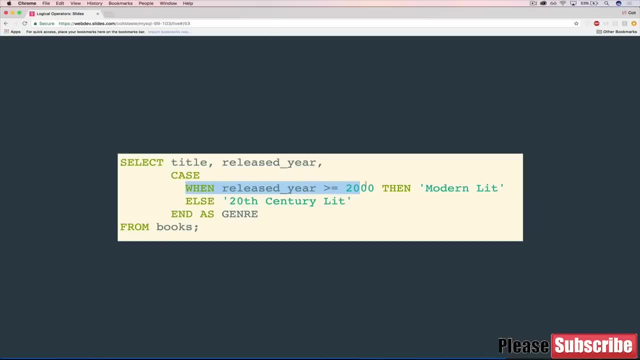 when released year is greater than or equal to 2000. then return modern lit, and when I say return it's a programming term, but basically means spit out. think of it as just making genre equal to modern lit. so that happens when released year is greater than or equal to 2000. 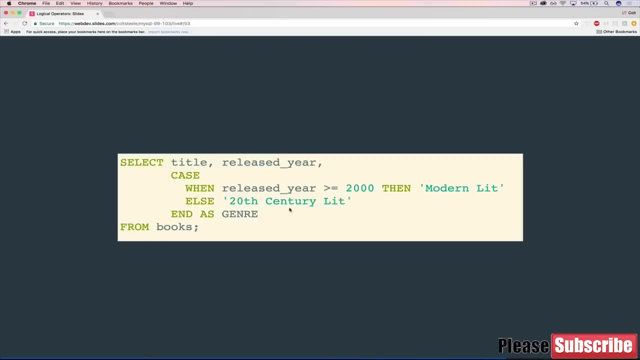 then we have an else which is otherwise. we're going to return 20th century lit. so this is basically saying if it's greater than 2000, if it was released in the 2000s, then make genre modern lit. otherwise it was released in the 1900s. 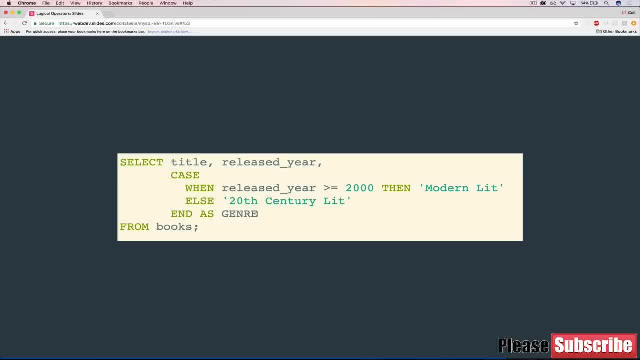 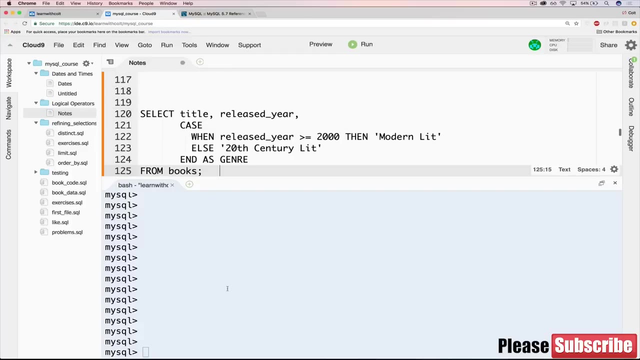 so we're going to print out 20th century lit for genre and that's how we end up with this. so we have this bit of conditional logic where genre changes depending on the value of released year. so let's actually try this now. run it and you can see. 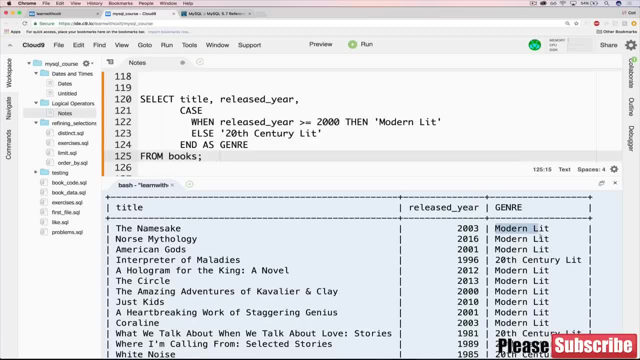 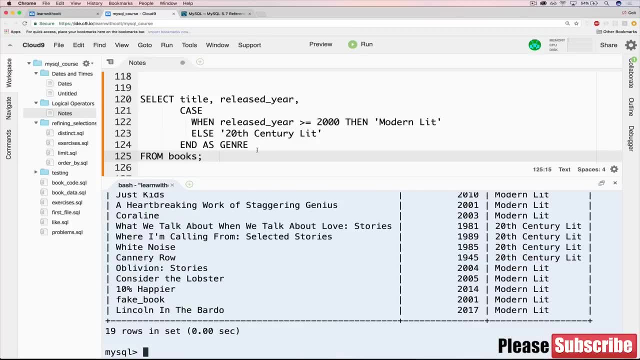 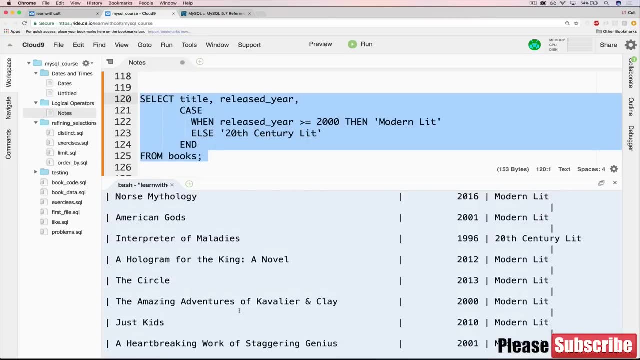 we get the namesake. 2003 is modern lit. interpreter maladies, however, is from 1996. so we get 20th century lit and I will show you if I get rid of the, as it's a nightmare because if you look at what we have as our, 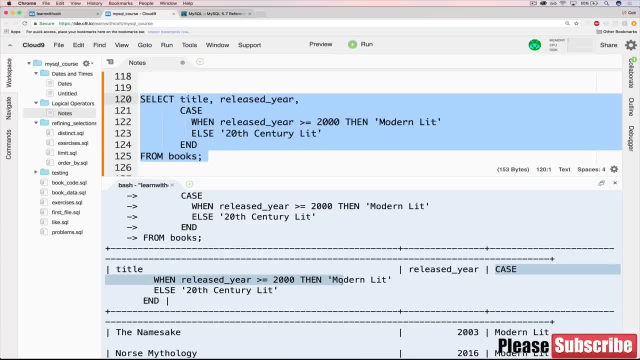 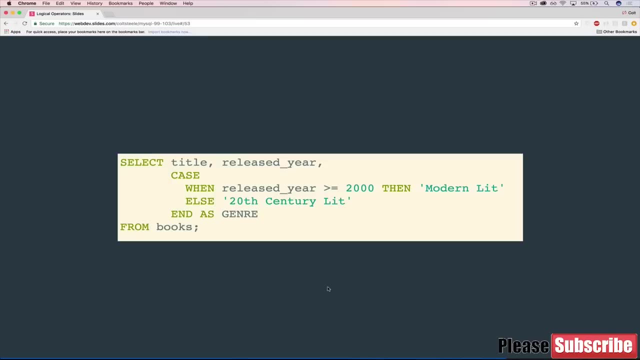 headers. here we have title, release year, and then we have case when released greater than 2000, then modern lit, else blah, blah blah. so you definitely want to use as when you can. ok, so that's one example, but I do think this one benefits from a couple, because it's a bit weird. 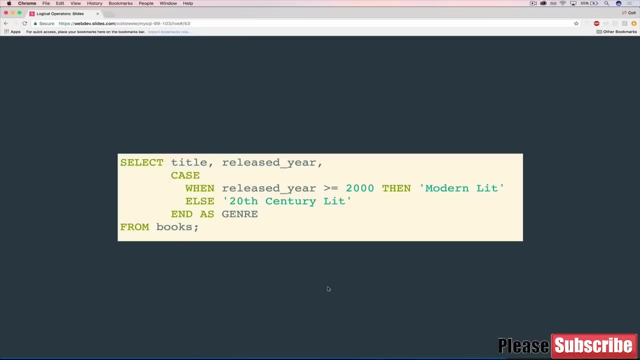 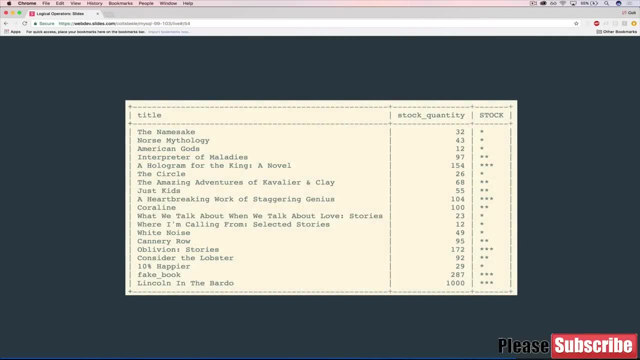 especially if you don't come from a programming background. so don't panic if you're not comfortable with this type of logic, but if you are, it's very similar. if you're not, it's kind of a new, a big new idea. so here's another one. 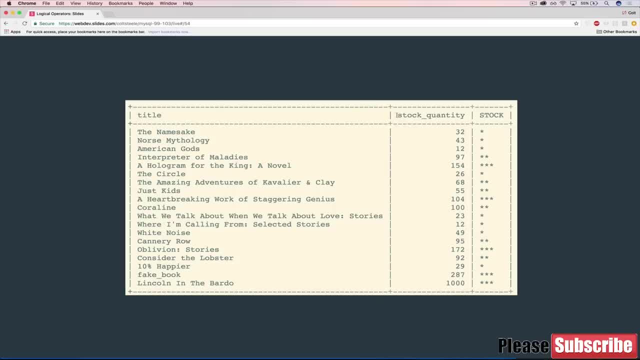 what I've done here: printed out title and then stock quantity, and then I'm using stock quantity to then print a graphical representation of how much stock we have. so one star is things that are lower in stock, two star has a medium level of stock and three stars means we have a lot of stock. 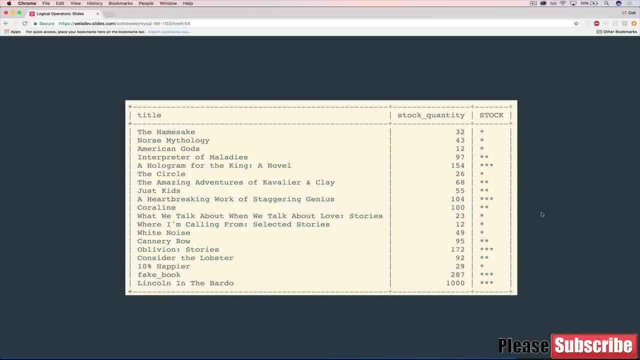 and I can't remember the exact numerical breakdown where that happens. I believe if it's 0 to 50 copies, we have one star, if it's 50 to 100, we have two stars, and then, if it's 100 or more, we have three stars. 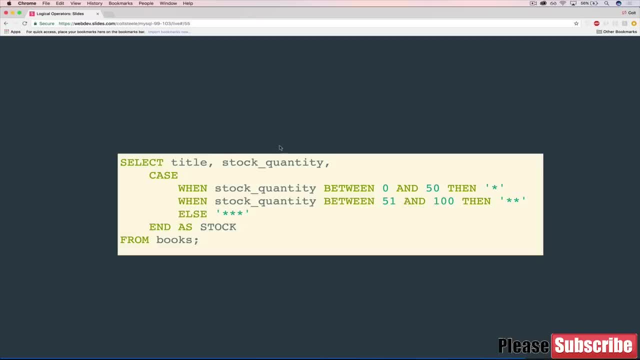 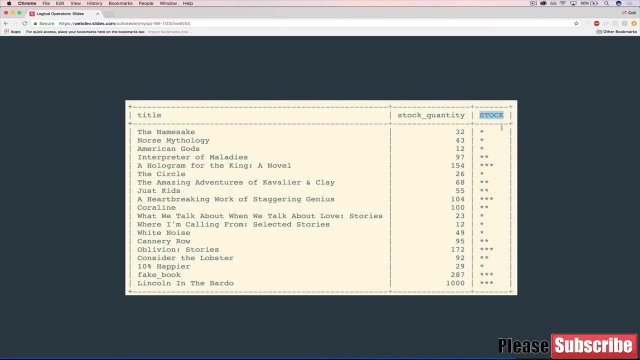 so it looks like this. so let me show you select title and stock quantity from books. again, beginning and end is the same. then we have our case and then the end of the case with this alias stock. so that's just going to give us stock right here. 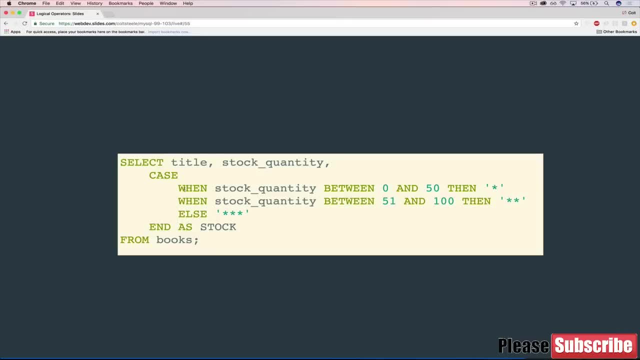 and then the important part. so when stock quantity is between 0 and 50 and we don't have to use between, we could use what we saw earlier, our logical, and we could say: when it's greater than equal to 0 and stock quantity is less than, 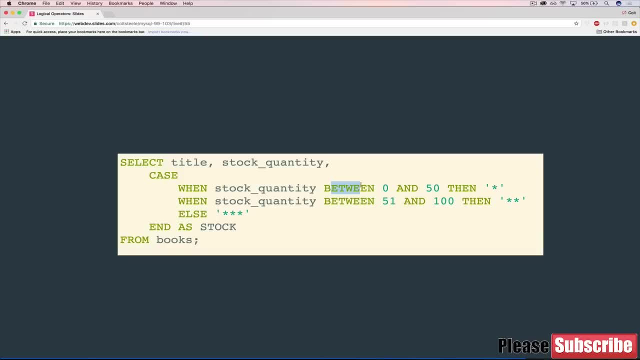 50, then blah, blah, blah, but it's much easier to use between. so when stock quantity is between 0 and 50, then stock is one star. so that's how we end up with one star. but if that's not true, then it moves on to the next one. 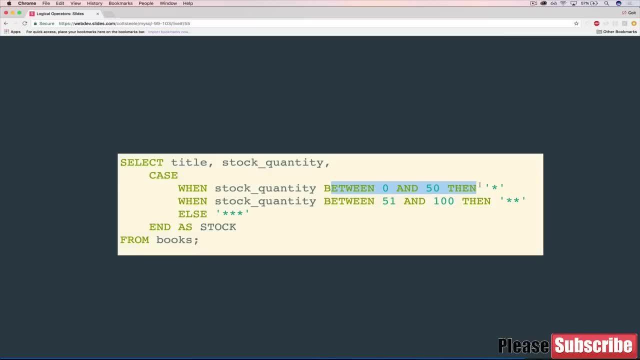 so if stock quantity is 100, this is false, so it ignores it and it tries this. well, is stock quantity between 51 and 100? if it is, then stock is going to be two stars, and if it's greater, let's say it's 153. 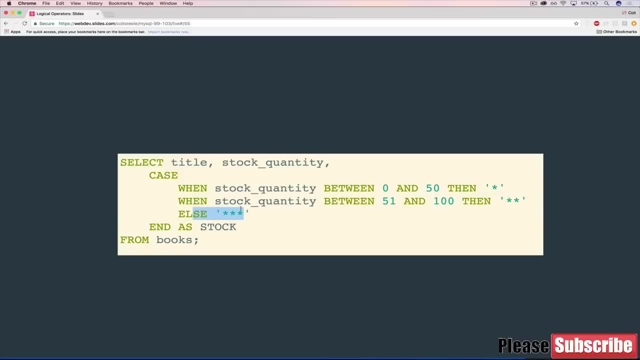 well, this is false, and this is false, so it goes to this. last one else has no other choice. this is otherwise. if nothing else above was true, well then, this one is three stars, so it goes through. and it does that for every single one, so we end up with one. 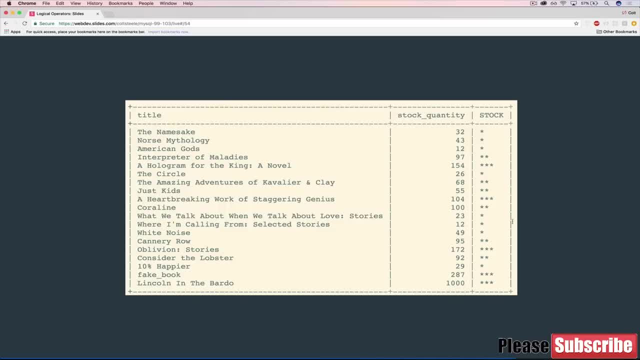 two and three stars, so hopefully you're getting the idea here. it's pretty powerful. it allows us to make decisions or do have different outcomes, depending on our data. one thing I definitely need to point out, because I can see this as being confusing: you don't have to have 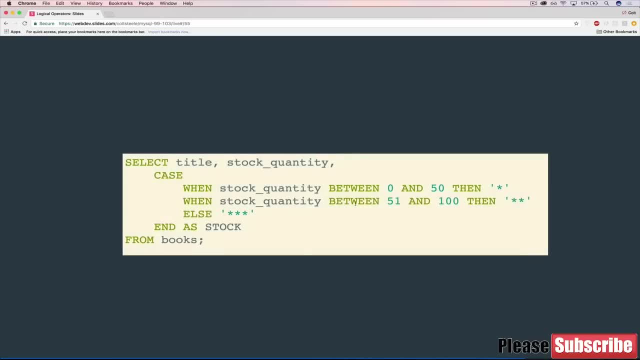 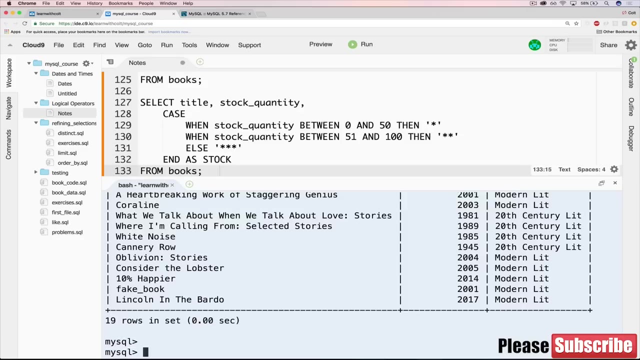 stock quantity printed out in order to reference it in your case statement or back here. I don't have to work with release year up here in order to work with it in the case statement, so let's actually copy this one over and run it. make some space. 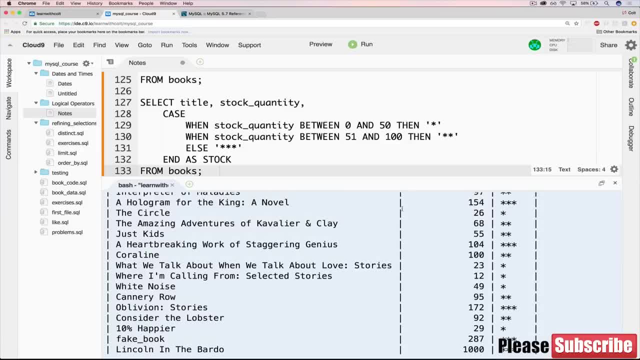 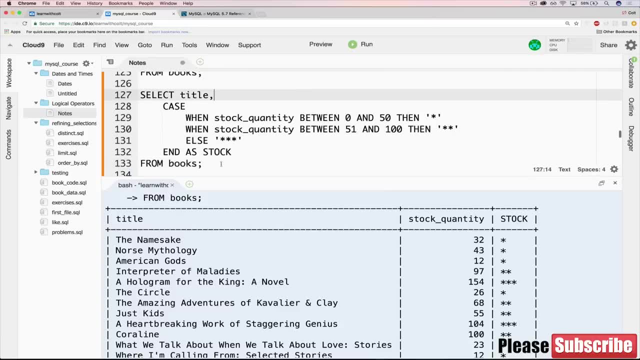 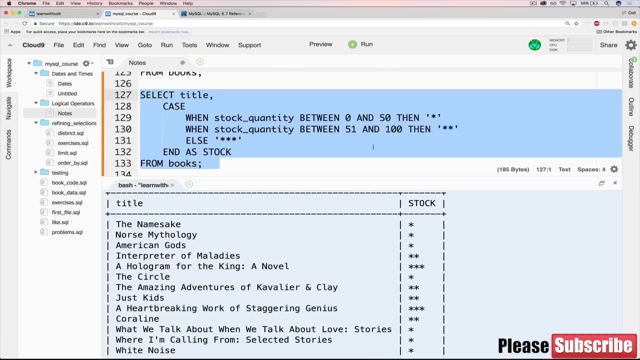 here we go. okay, so we see the same thing. but just to show you, I'm not going to use stock quantity up here, I'm just going to select the title and our stock visualizer and there we go. so I just wanted to show you. you don't have to have. 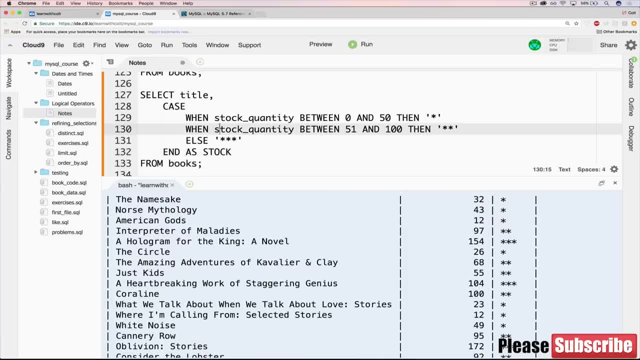 stock quantity referenced in order to use it inside of your case. and another point I should make is we're not limited in this number of how many conditions we could have, so if we wanted to, we could have another one here when stock quantity is between 101 and 150. 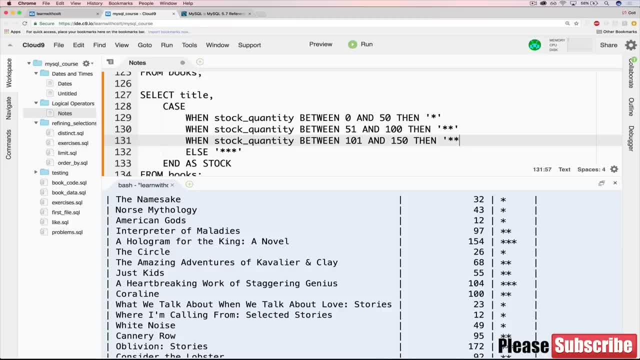 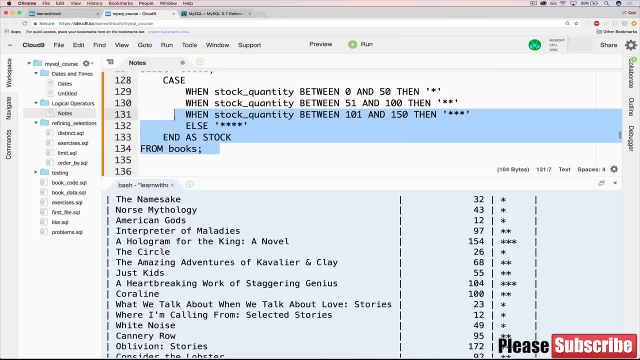 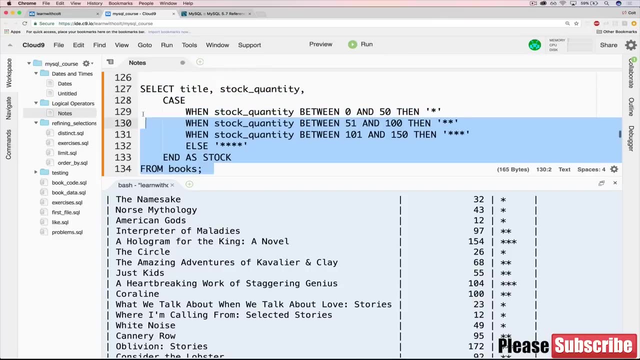 let's say then it's 3 stars, otherwise it's higher than that. so we'll say 4 stars. so let's try that. let's actually add stock quantity back in- it makes sense to be able to see that- and let's copy it over and run it this time. 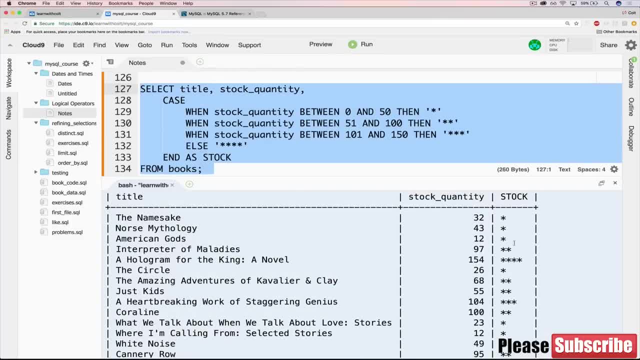 and now we have 1 star, 2 star. we've got 4 stars for 154 and 3 stars for 104, so my point is that you're not limited. another thing that trips me up personally is I'm inclined to put commas here. 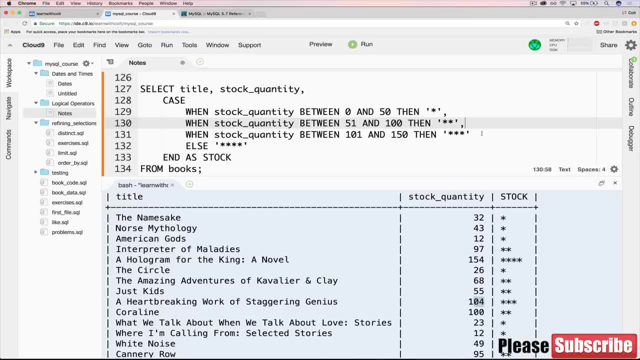 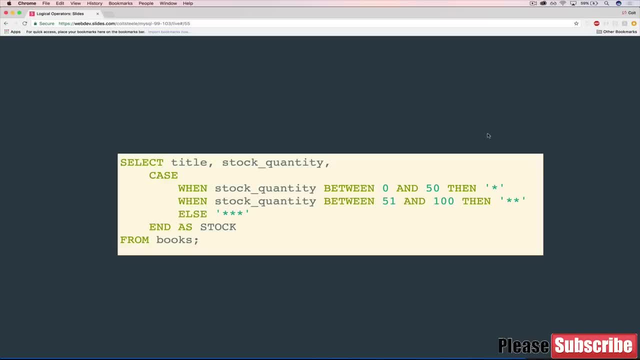 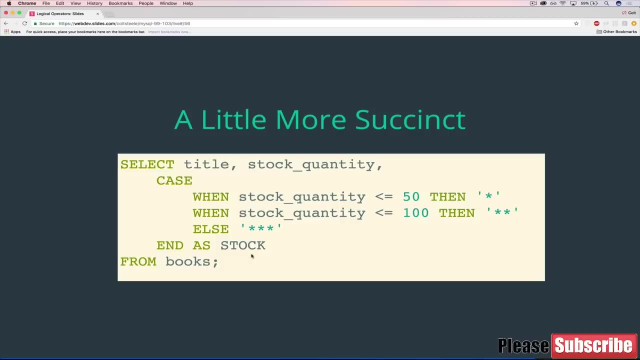 just because most things in MySQL are separated by commas. if you have a list of values or a list of anything, that will break it. so no commas there. so let's try that, ok. so one other thing I did want to address is that we could make it shorter. 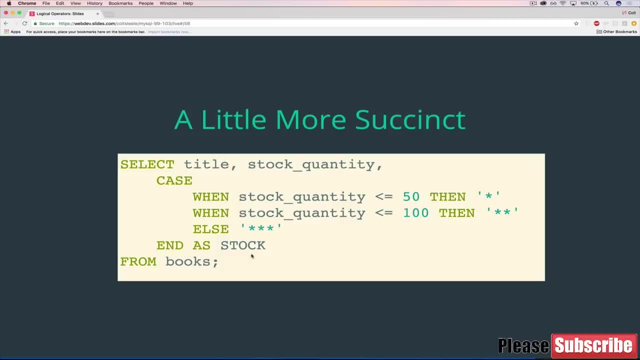 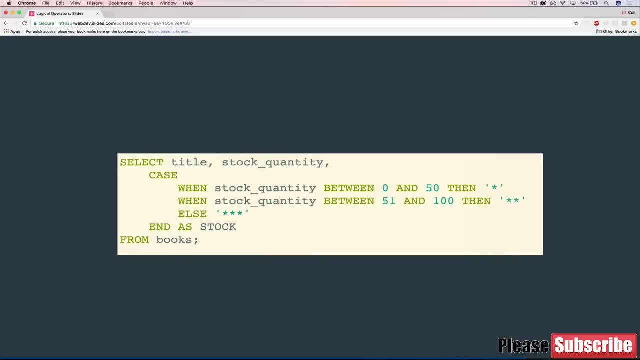 if we don't use between and, the way that we can do that is by taking advantage of the execution order of things. so let me show you. here's another, the same exact outcome as this line of code, where we have 1,, 2, and 3 stars. 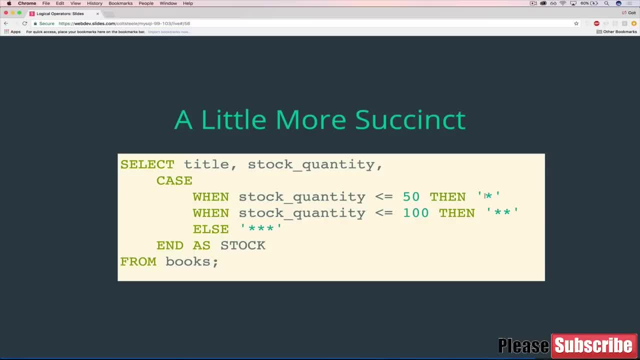 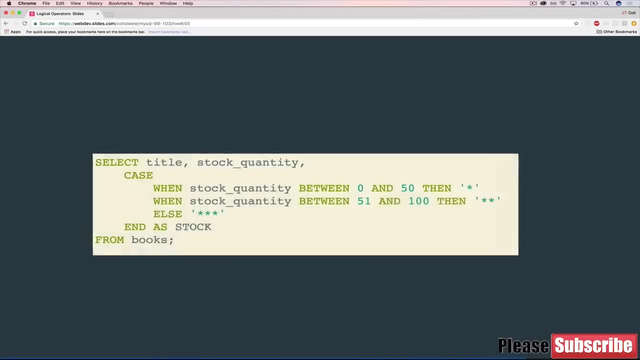 however, it's much shorter because what's happening here? so if it's less than or equal to 50, that means already it's greater than 50. so if this line is running, we know for sure stock quantity is greater than 50. they go in order. 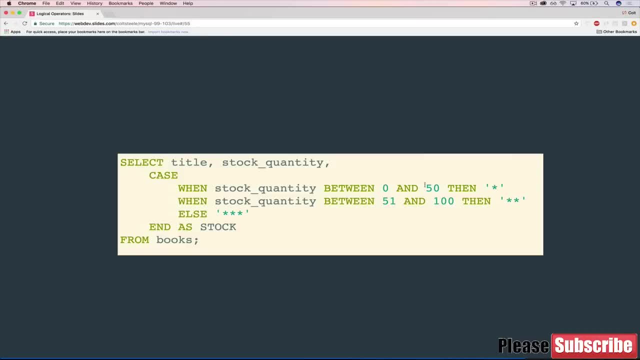 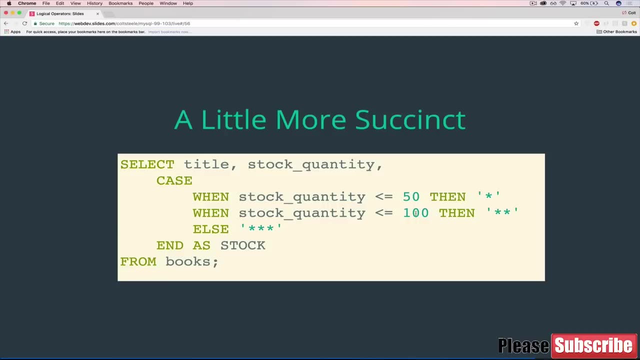 so we don't have to necessarily add this between, because we know, alright, it's definitely greater than 50, so we can just take advantage of that and just say, ok, well, is it less than or equal to 100, which is the equivalent of saying: is it between 50 and 100? 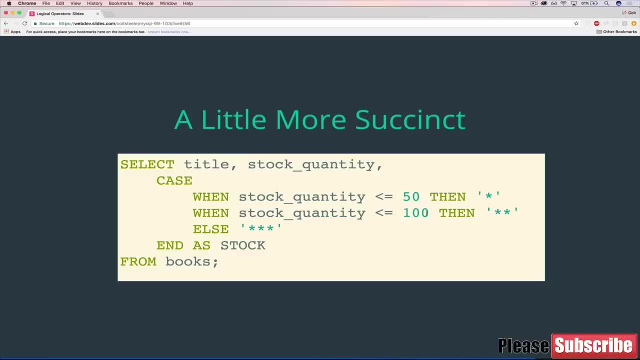 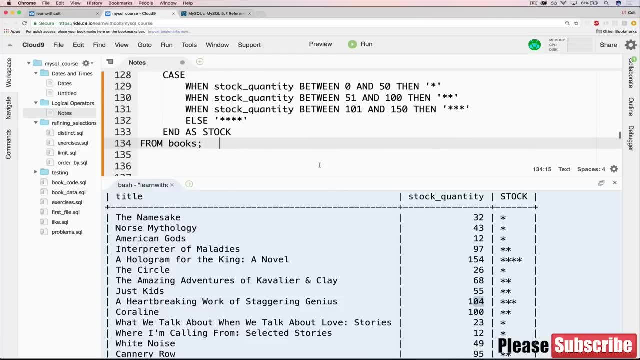 if it is, then it's 2 stars less than or equal to 100. then that means it's greater than 100, and so we get 3 stars. so this is more just showing you a way of cleaning it up, if you wanted to, so you don't have to use between. 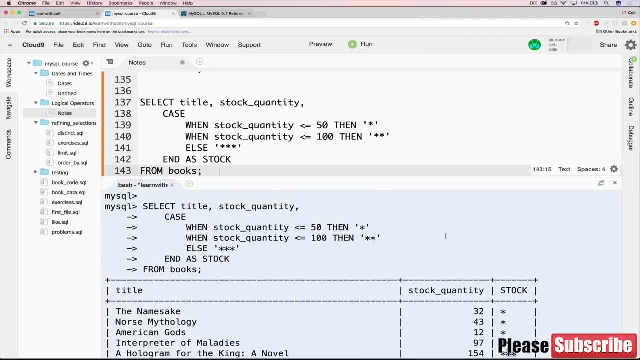 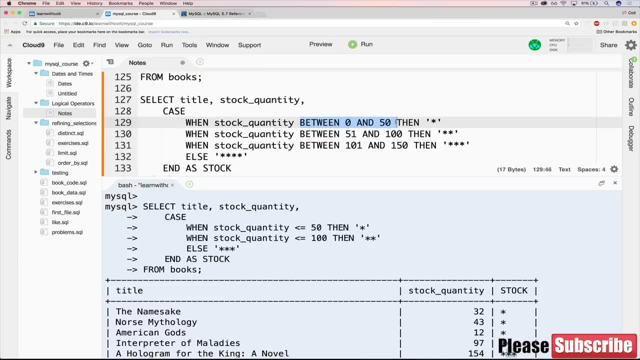 and you can see we get the exact same outcome. 1,, 2, and 3 stars. we don't have to use those longer between statements, although some people would argue between is easier to read, it's more semantic, more understandable when you look at it. 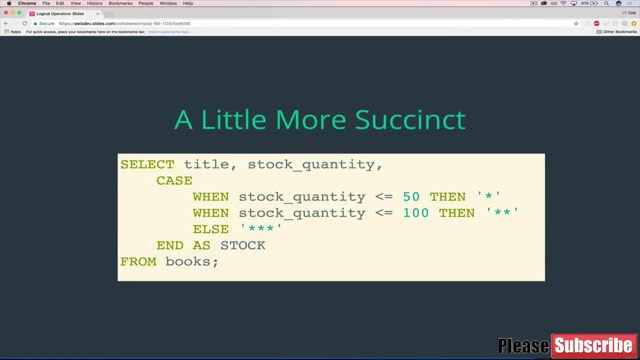 rather than working with this. so that wraps up this section on case statements, which hopefully you see what I mean when I say they're both very useful but possibly a little intimidating, especially syntactically. there's a lot there, so definitely take some time on the next couple of exercises. 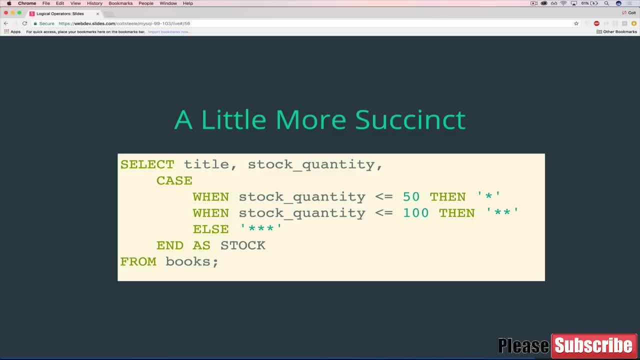 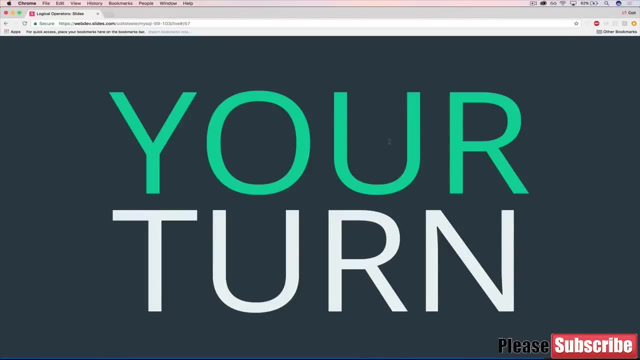 I'm going to have a few that require you to write case statements. hopefully you'll get some practice there and you'll see how powerful they are. with that said, we're moving on to exercises. alright, so you probably guessed it either. in the last video I told you. 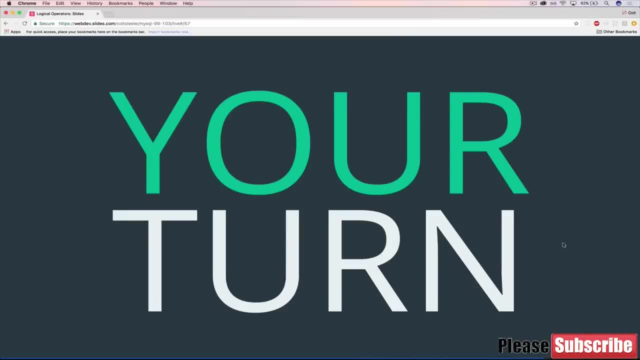 or because of this gigantic text. here it's your turn to try putting this into practice. so we got a couple of exercises. they range from trivial, simple logic questions all the way up to more complex case statements, so I encourage you to go through all of them, especially the case statements towards the end. 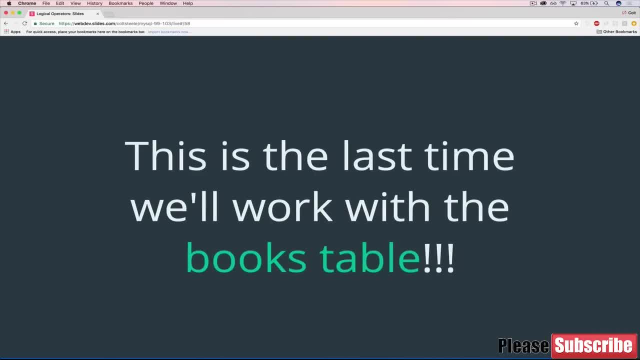 but hopefully you don't lose interest before then. oh, and one thing: this is the last time you have to work with those darn books. last time that books data. you can definitely play around with it, but I'm getting pretty sick of it. I imagine you are, and the good news is: 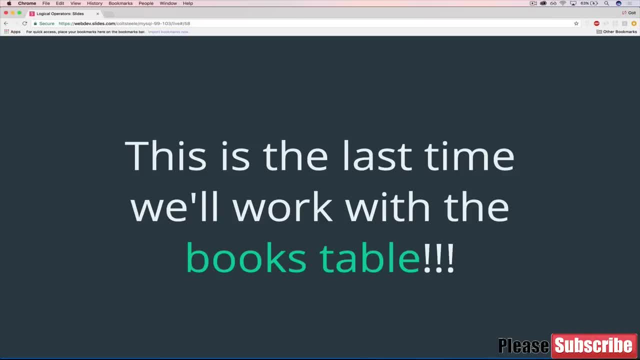 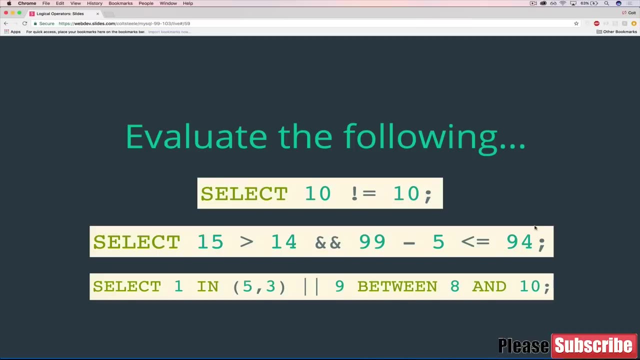 we're now moving on to join tables, which allows us to get much more complex and real life data, things that are more accurate and realistic, and that's really exciting. so get excited if you're not, alright. so here's the first couple. evaluate the following now. try doing them, don't just copy them. 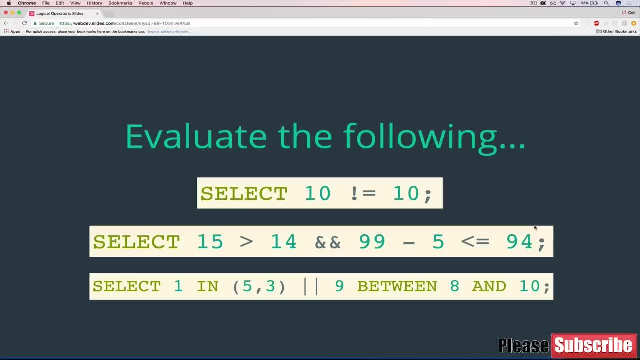 and paste them in and hit enter. actually walk through and evaluate. the result is so. the first one: select 10, not equal to 10. is that true or false? 0 or 1? next, select 15 greater than 14 and 99 minus 5. 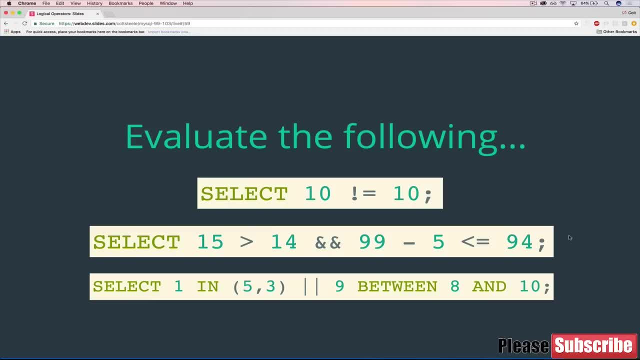 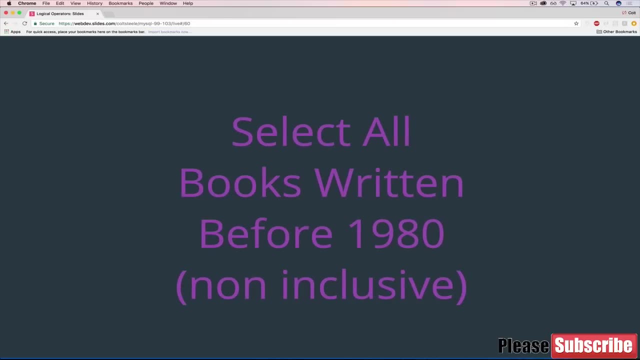 less than or equal to 94. true or false. 0 or 1. finally, select 1 in 5 comma, 3 or 9, between 8 and 10, true or false. so do those and then move on to these code based challenges. so the first one here is: 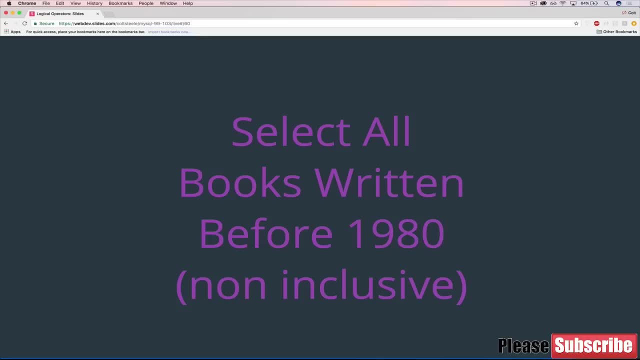 select all books written before 1980 and that does not include 1980, so everything up to 1980, but not 1980. once you've done that, move on. I've got some beautiful red text really expanding the color palette. select all books written. 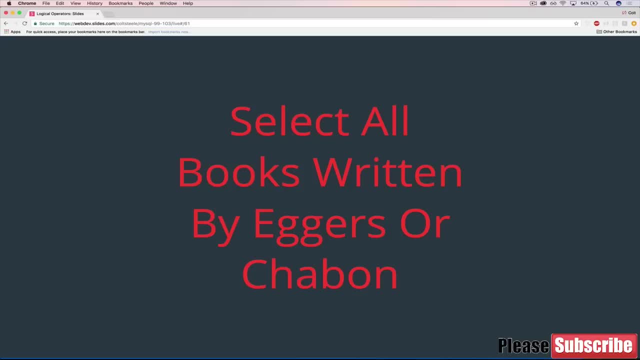 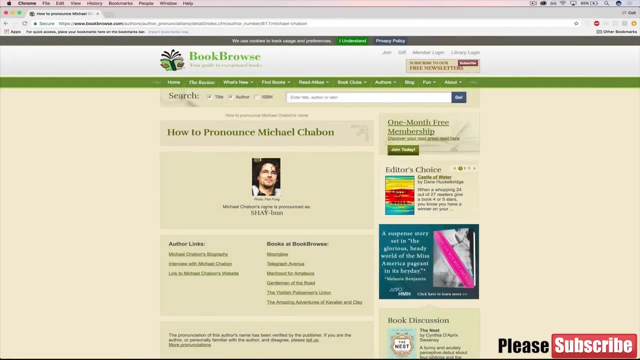 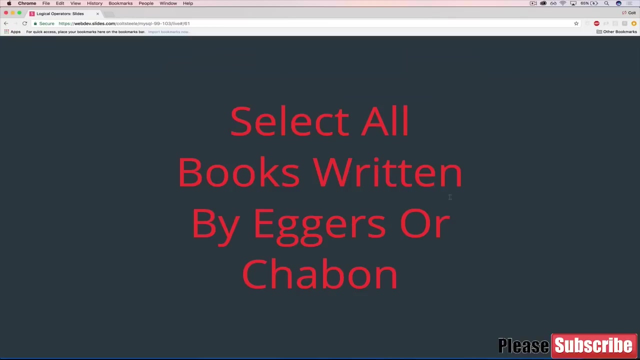 by Eggers or Chabin. I don't know how you say his name, honestly, that guy great author. well, I just googled it and apparently it's pronounced Chabin. so select all books written by Eggers or Chabin. makes sense, now that I think about it. 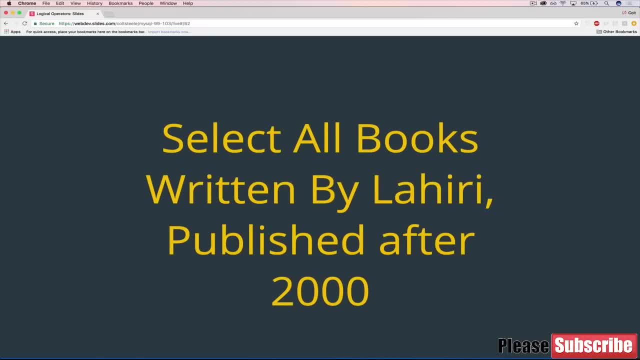 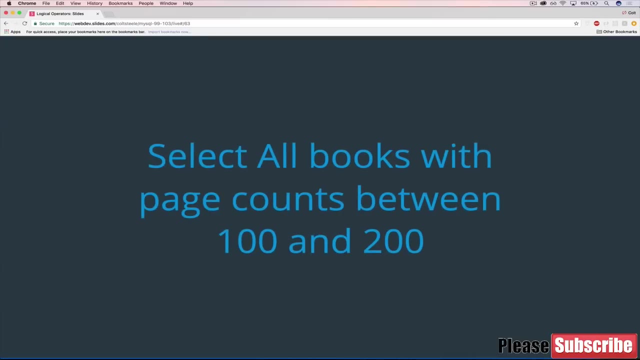 now onto the beautiful yellow. select all books written by Lahiri published after 2000, so books written by Lahiri released after 2000. then select all books where the page count is between 100 and 200 pages, so our middle length or short books. those are pretty short. 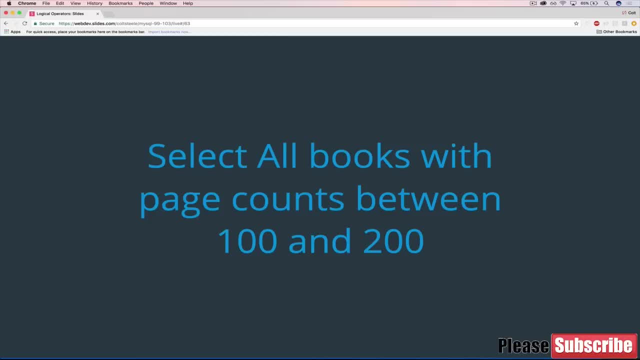 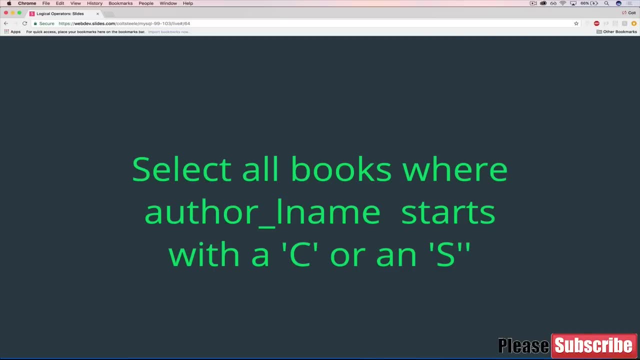 between 100 and 200 pages. next, select all books where the author last name starts with a C or an S, so this one. there's a couple of ways of approaching it. I'll let you discover what works best you may want to use. well, you'll need to use things that we've learned in the 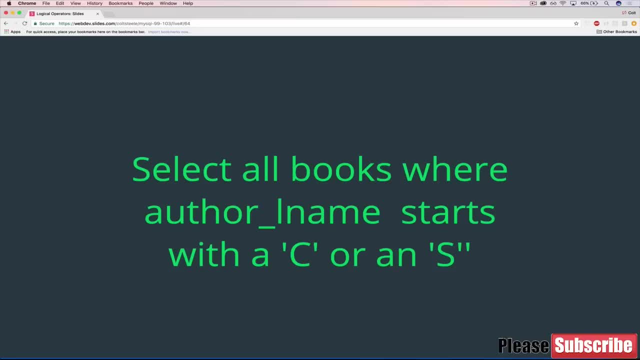 past, especially when we're working with string, so you may want to go back or just go to the string documentation to figure out how to do this. select all books where the author last name starts with a C or an S. those are my initials, so maybe I'm crazy and I just want books that. 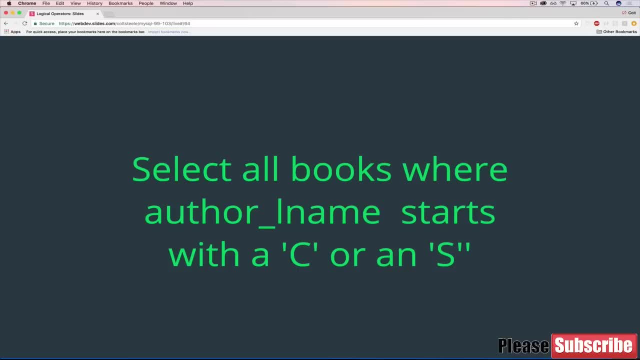 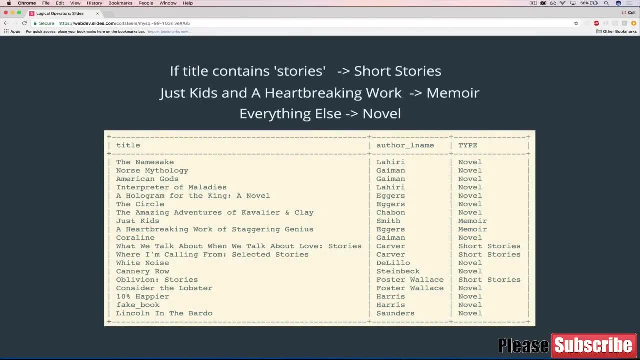 start with, who are written by authors who start with my initials- I don't know. now moving on to the main event, our wonderful case statements. so here is another example. this is done using a case statement and let me explain it. so we've got title and the author last name. 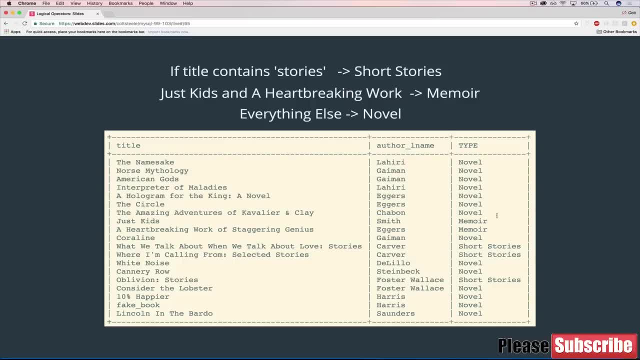 then we've got a type over here. what type of book is it which? I'm really bad at this? this should just be called genre. it doesn't matter, though, basically the way that it works, if the title contains the word stories, we're calling it short stories. 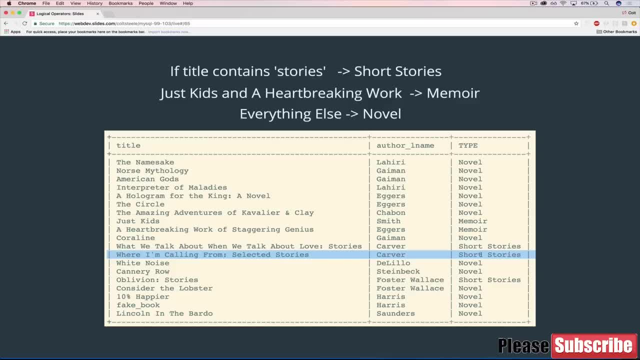 so, as you can see where I'm calling from, selected stories is categorized as short stories. what we talk about when we talk about love great collection is categorized as short stories because it contains stories. same thing with oblivion stories. then there's another part if the title is just kids. 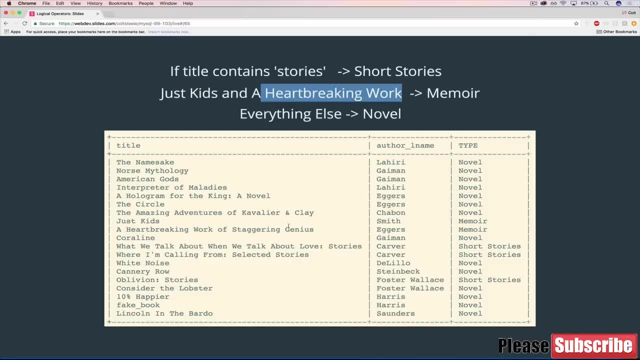 or it's heartbreaking work of staggering genius, which I didn't write all the way up here because it's giant. but basically, if it's this book or if it's this book, both are memoirs. so we have these two exceptions that you'll need to write in. 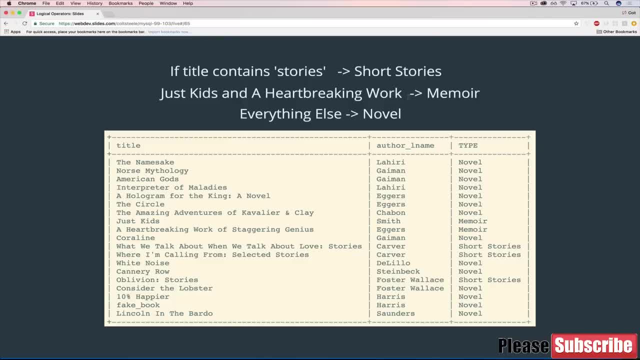 finally, everything else which hopefully sounds familiar. otherwise, everything else at the end is called a novel and I know some of these aren't actually novels, like consider the lobster. it's more of an essay or collection of essays. 10% happier is like a self-help book. but I didn't want. 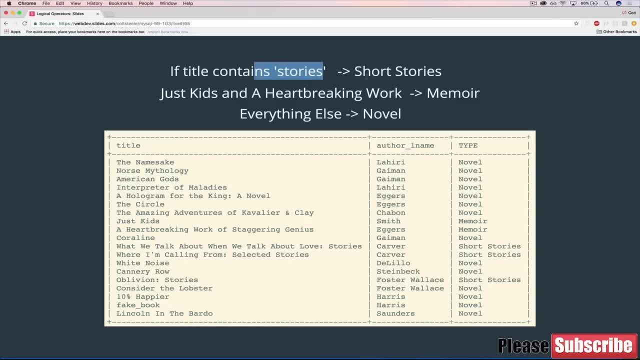 to get too complex. so just to reiterate: the title contains stories. type is short stories. if the title is exactly just kids or exactly a heartbreaking work of staggering genius, then it's memoir- both great memoirs, by the way. and then finally everything else is a novel. okay, 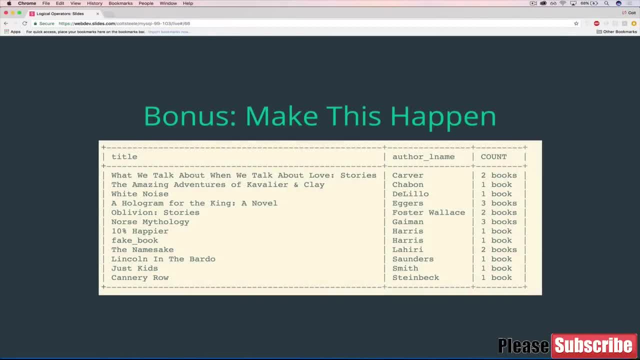 one more. this is a bit of a bonus, so it's more complex. you have to put a few things together, so we have title of the book and the author last name once again, but then there's this count section and count, which we've already seen how to do. 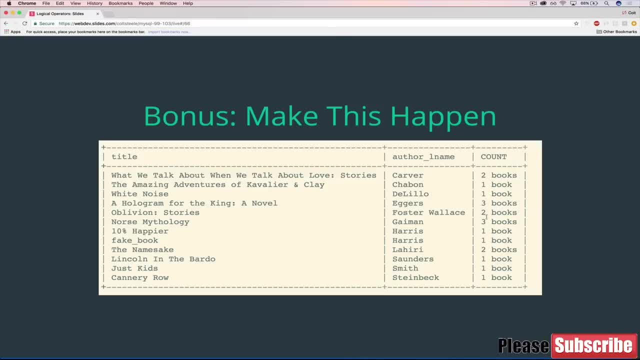 is a little different. it's not just saying two or one or three what it's actually doing. we can ignore the title part. actually, you don't need to do that. just focus on the last name of the author and the count. it's saying how many books each author has. 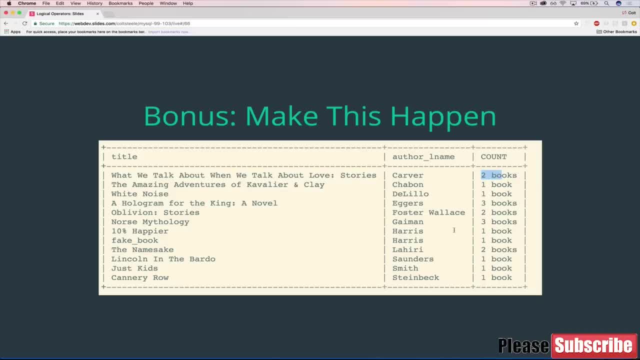 how many they've written. so Carver has two books, Hayden has three books, Harris, Dan Harris or Frida Harris. they each have one book. Jubilee here, he has two books, and so on. but not only is it printing the number, but there's also the properly pluralized. 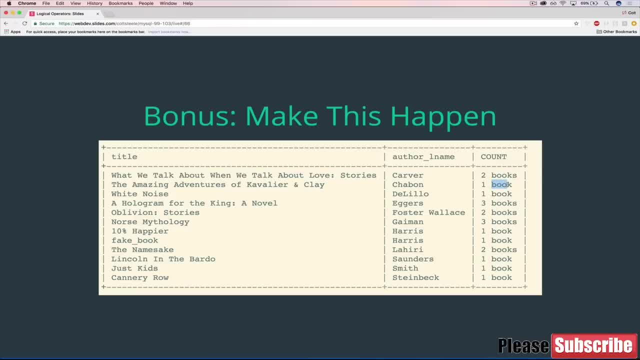 books or book following it. so one book, singular, two books, three books, one book, and so on. so you'll need to use a couple things. I can give you hints. if you don't want the hints, then stop right now. but the hints are you need to use group by. 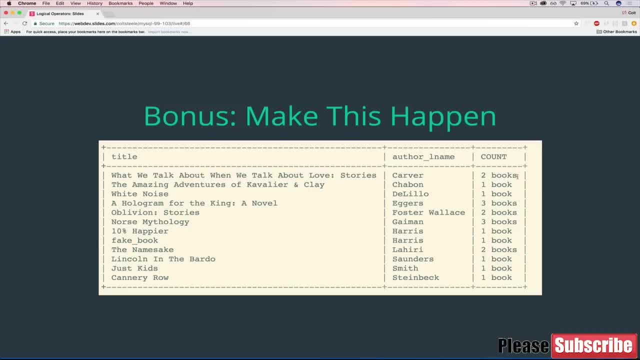 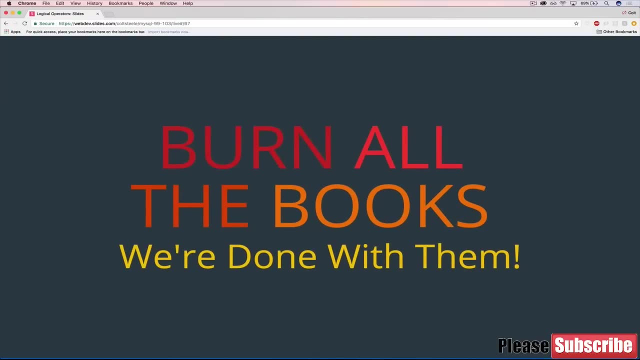 group. you need to also use a case statement to generate this right here, but it is a bonus because you do need to combine a couple things. it's a decent amount of work, okay, so that's it. once you finish that, burn all the books, we're done with them, whatever that means to you. 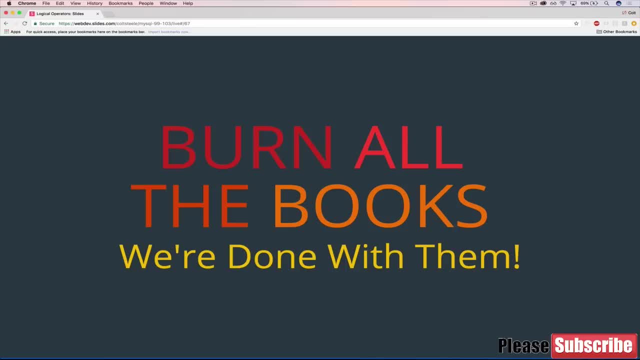 I don't actually condone burning books, but if you want to get rid of the database, go ahead. although you may want to refer back to it, this is more just me saying that we're done- done with the books. this is a turning point. we're moving on to some bigger and better. 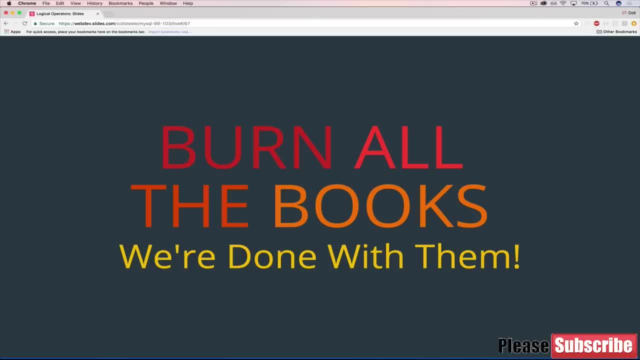 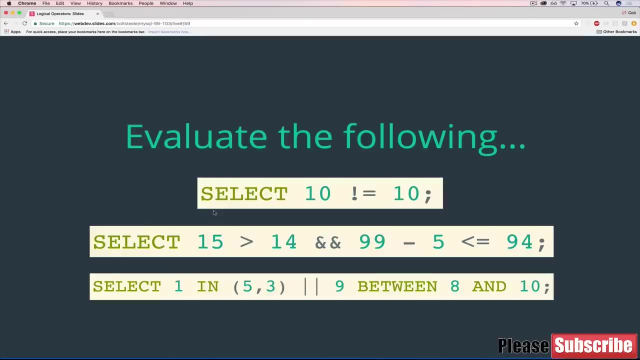 data and to pretty important section which is joins. so I definitely recommend you take a break, but I will reiterate that in the solution video which is coming up next. okay, so let's go over. hopefully you're still alive. it was maybe a bit of a challenging problem set. 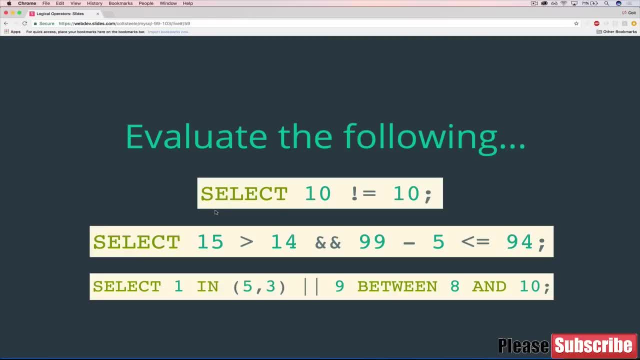 but if you're still here, let's go with these first three. so evaluate the following: select: 10, not equal to 10. well, 10 is equal to 10, so this should turn false. we get 0. next one a little more complex, we've got an, and so remember that means. 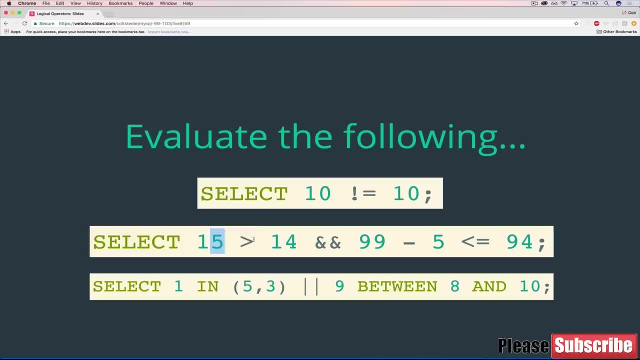 both sides have to be true. start with the left. is 15 greater than 14? yes, so that's true. but how about this side? 99 minus 5 gives us 94. is 94 less than or equal to 94? yes, it's equal to. 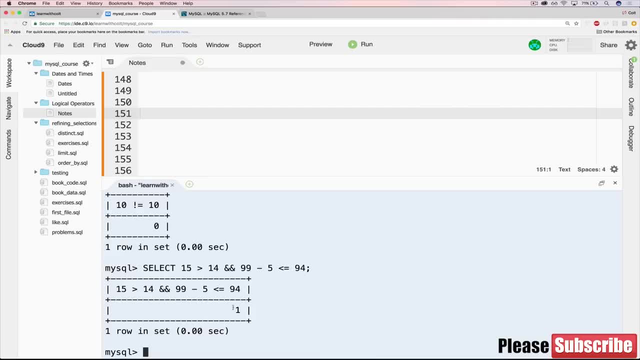 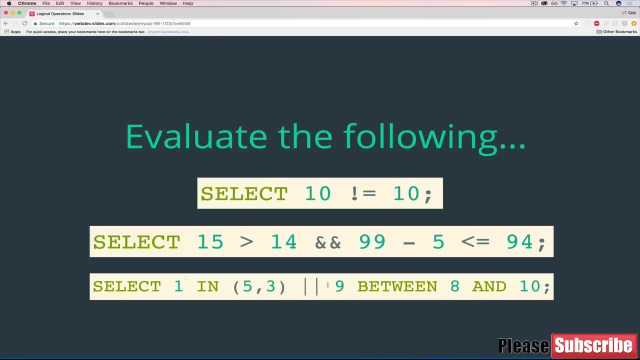 so that means both sides are true, meaning the whole thing is true. which we get, 1, finally select 1 in, or 9 between 8 and 10. so we've got, or either side can be true to make the whole thing true. so let's start with this. 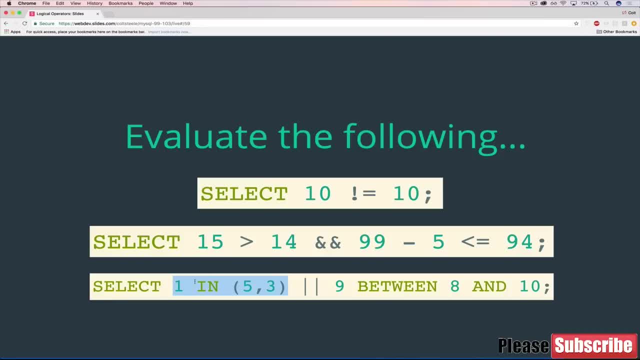 select 1 in. remember this is. I didn't show you this explicitly, but we saw how to use in so you should know how it works. is 1 in that set of no? so this side is false. but that doesn't nullify the whole thing. it doesn't falsify it. 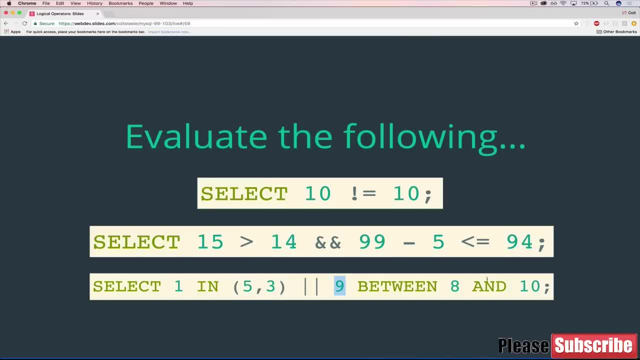 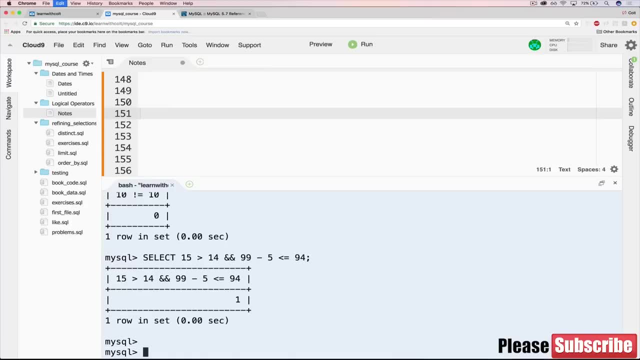 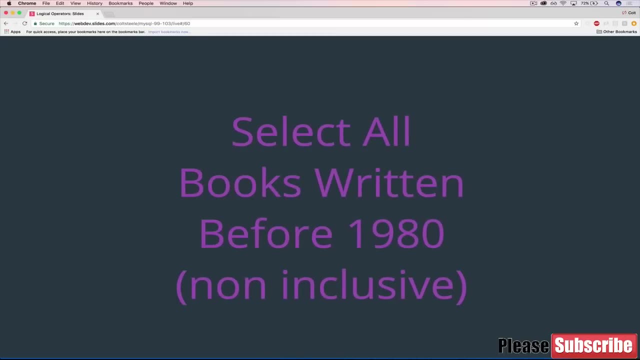 because what's on the right side is 9, between 8 and 10. yes, it is. so, this is true, making the whole thing true. let's try it. there we go, we get 1. so false, true, true. next, select all the books written before 1980. 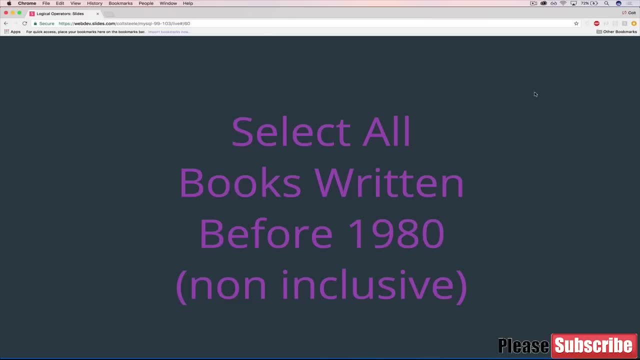 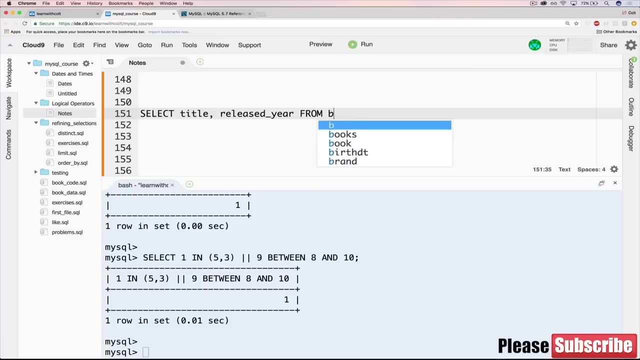 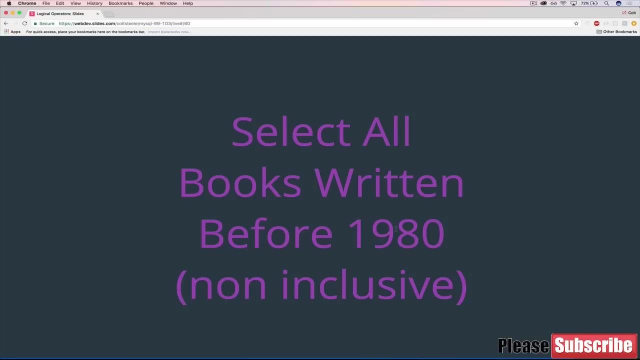 so I didn't specify what part of the book. that's totally up to you. let's just do title and released year so we can see that released year from books and then the key thing is we want to do where released year is less than 1980. 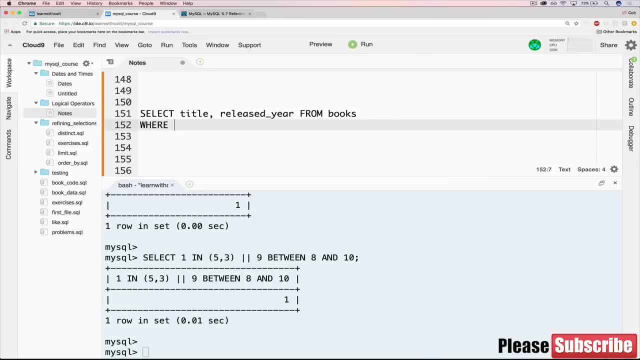 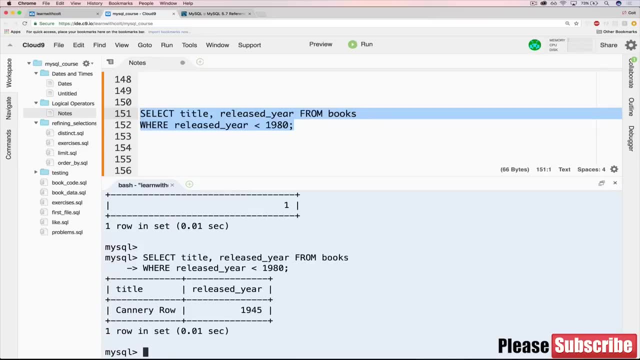 and not less than or equal to, because it says non-inclusive, so less than where released year is less than 1980. let's make sure it works. and there we go. all books written before 1980. apparently we only have 1. let's just. 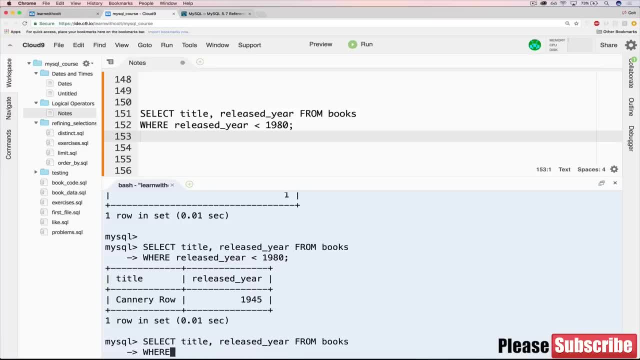 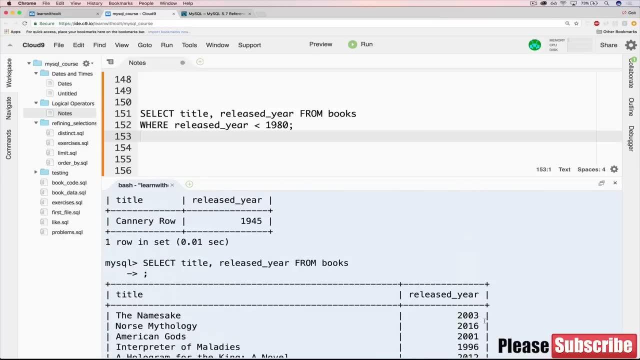 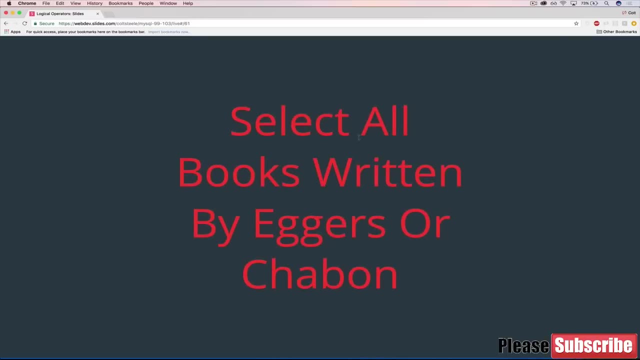 actually verify that. it's kind of catching me off guard there and it looks like that's the case. all we have is cannery row. well, I apologize, so we don't have more exciting data next up. select all books written by Eggers or Chavon. 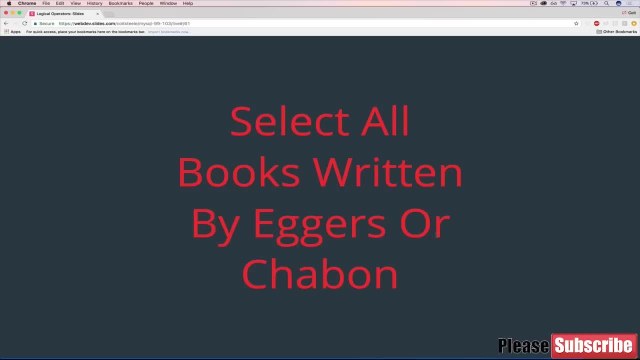 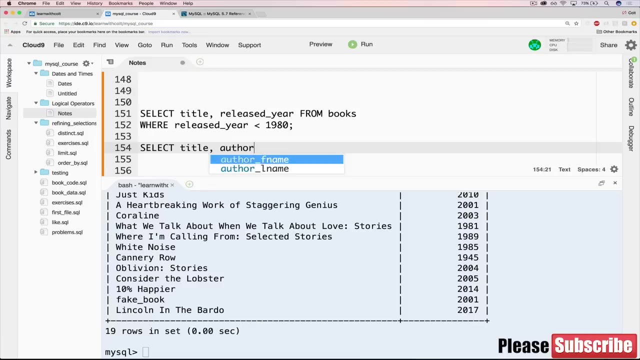 which I now know how to pronounce. so there's a couple ways of doing this. let's start with the most straight forward maybe, which would be, and also let's do title and author last name. so again, I didn't specify what parts you had to select, so 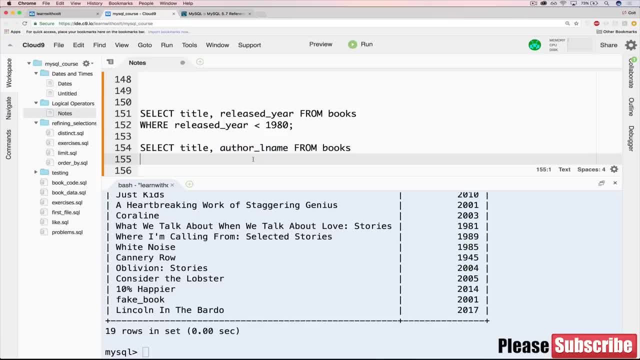 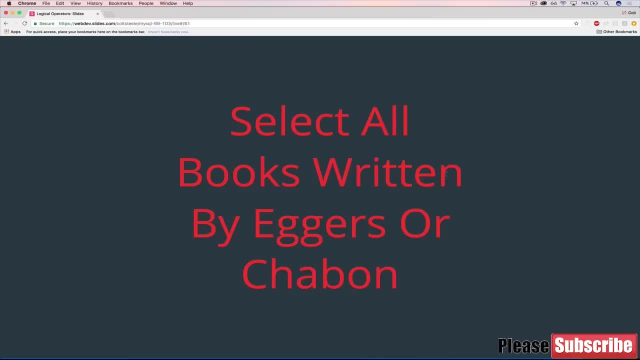 it's up to you, but this makes the most sense. so we can see the author last names. so what we can do is select them where and we can use an or, so we can do a double equality where author last name is equal to Eggers or author last name is equal to Chavon. 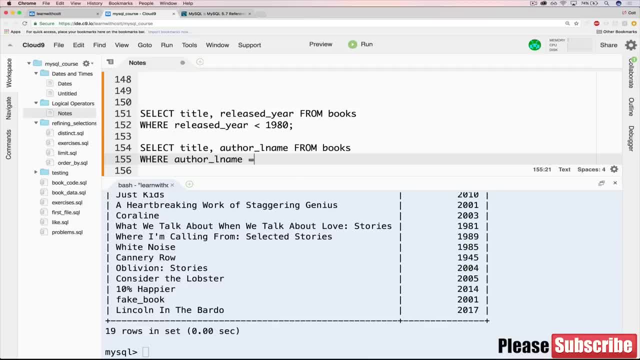 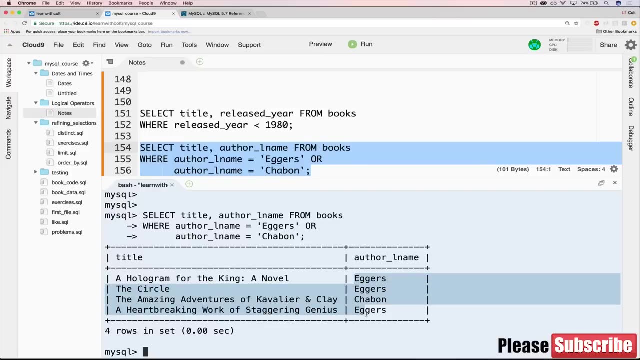 where author L name is equal to Eggers or author L name is equal to Chavon, just like that. that's one way of doing it and you can see we get those four books. however, we can also use in, because all that we're doing is trying. 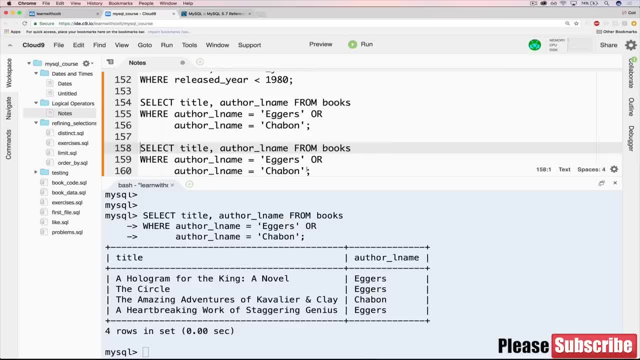 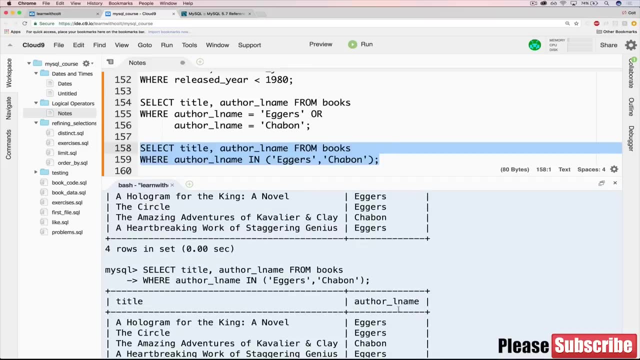 to see if author L name is in the set of Eggers and Chavon, so we can combine them, basically say where author L name in that set, copy that and there we go, same results. so whichever you prefer, this one is a little bit easier to see. 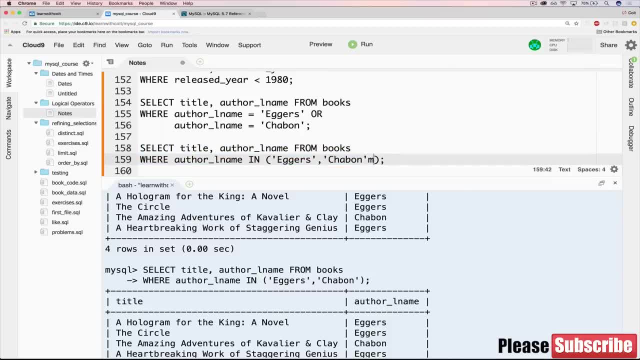 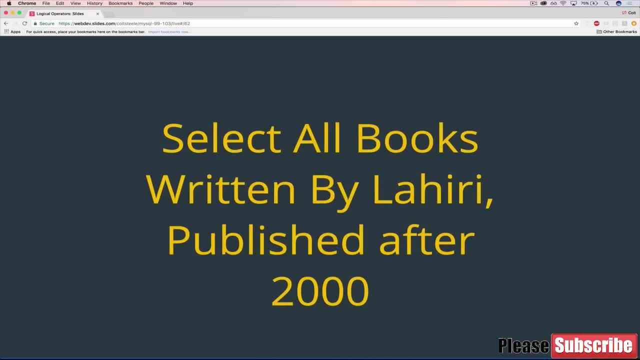 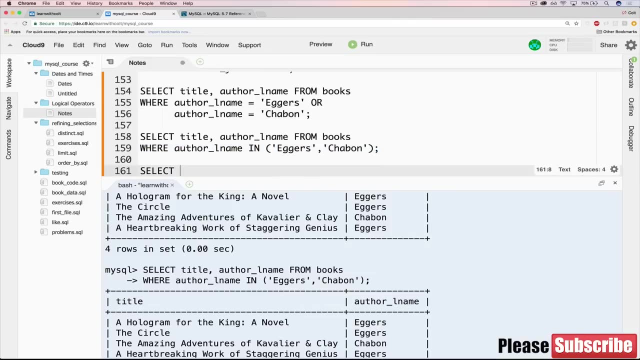 I guess it's shorter, easier to edit and if we wanted to add another author in, it's pretty simple. but this is also perfectly valid. next, select all the books written by Lahiri published after 2000. so the first thing we'll do title, and this time we'll do. 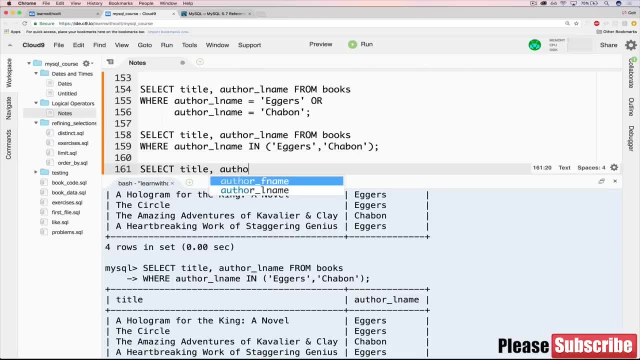 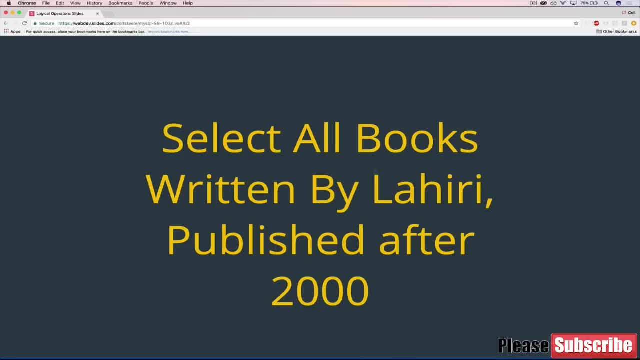 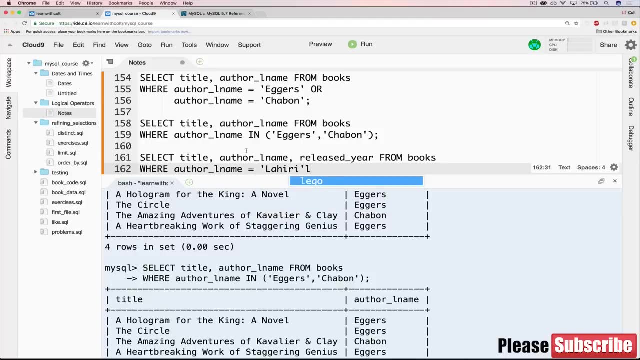 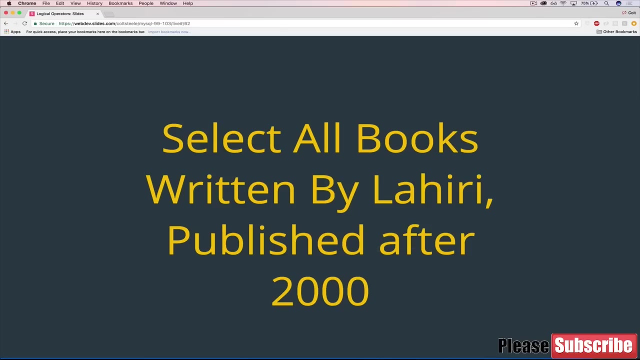 author L name and and released here from books, and we'll start by all books written by Lahiri, so where author L name equals Lahiri, so we can start there. we know this should work, but we get two books and now we want only the ones published. 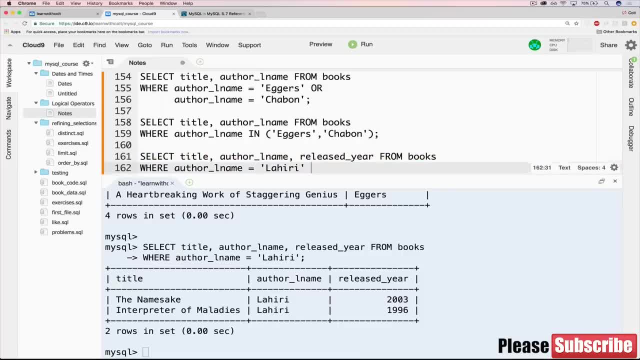 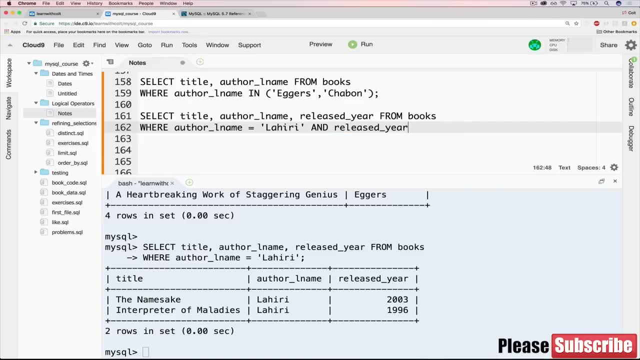 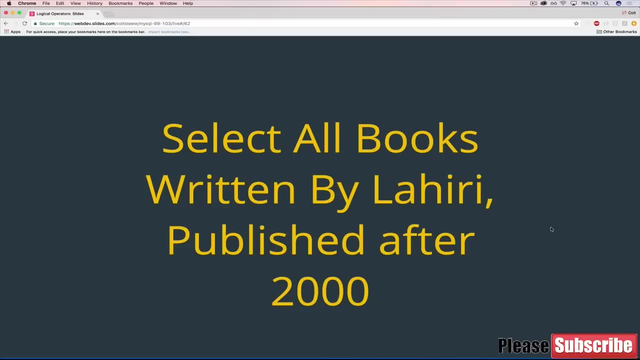 after 2000. so what we need is a logical, and so where author L name is equal to Lahiri and released here is greater than 2000- and I didn't specify if it was inclusive or not- so, based off the language published after 2000, we'll keep it as. 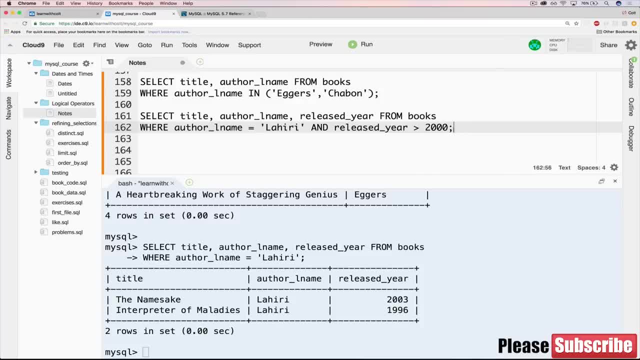 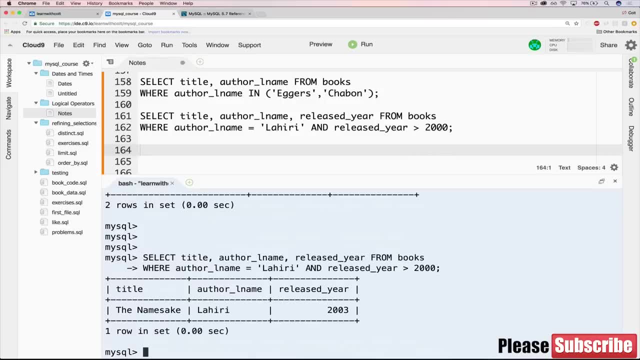 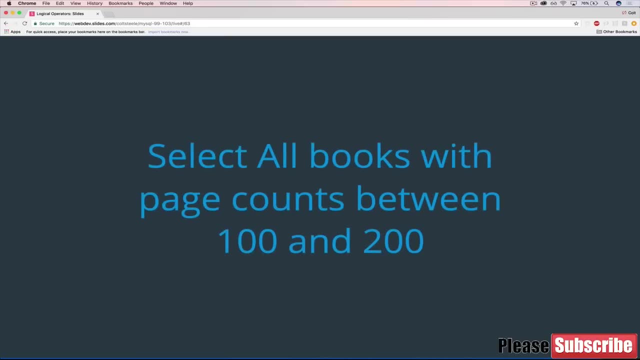 greater than if you put an equal sign there. it's not. I mean, you got it right essentially. I didn't do a great job of clarifying that before, so either one works. now we only get the namesake also really great read next up. select all books with. 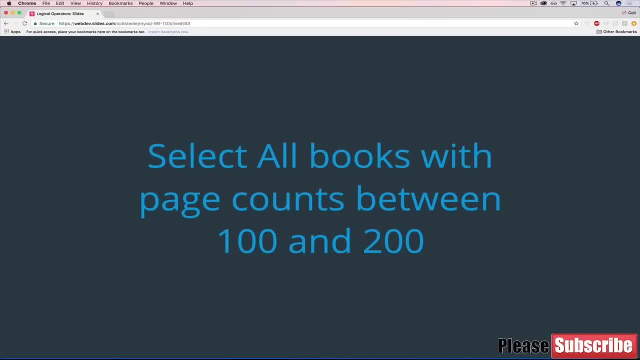 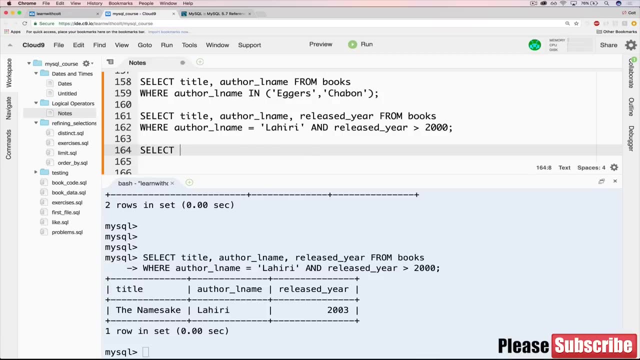 page count between 100 and 200. so, just like the problem we did back here, there's a couple of solutions. first one is to use logical, and so we can do select title and page count. or what is it? just pages from books where pages is greater than 100? 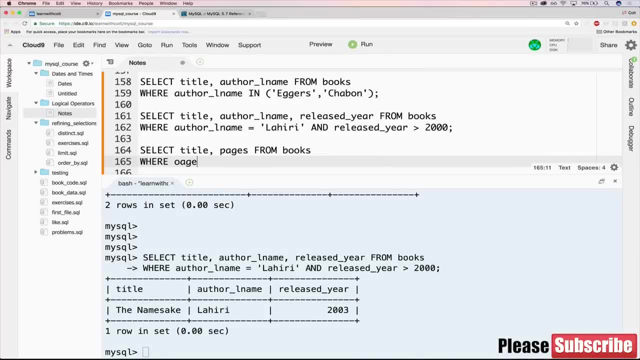 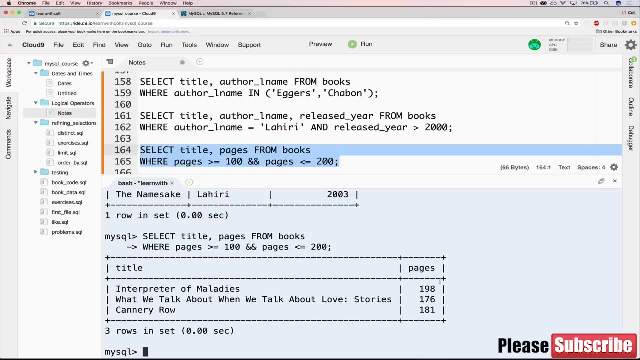 and less than 200, so where pages we'll do greater than or equal to 100 and pages is less than or equal to 200. that's one way of selecting based off of a range. there we get these shorter books, but we could also use between which maybe. 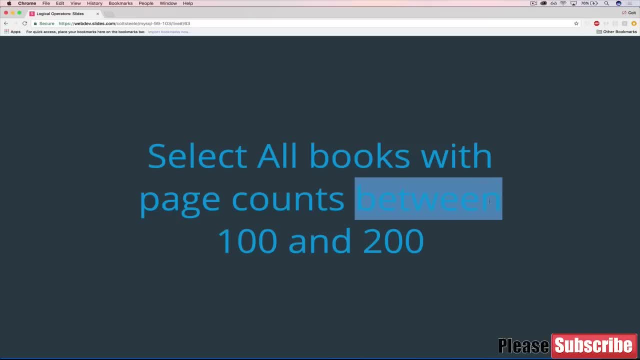 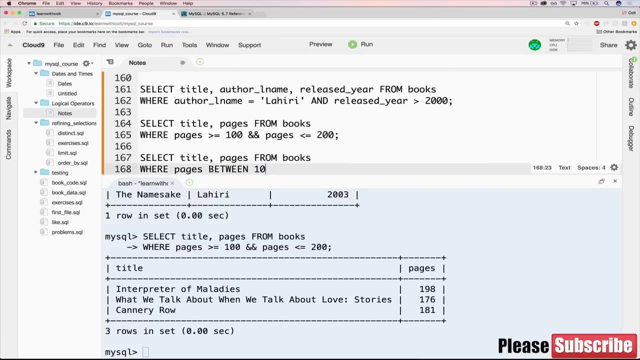 you gathered because of the language here it screams out between, and that might simplify it a bit. so all we have to do is change it to where pages between 100 and 200- nice, easy to read version. we get the same results. ok, one thing: remember that this is inclusive. 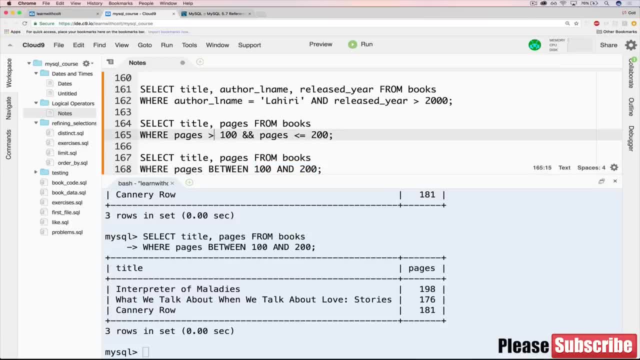 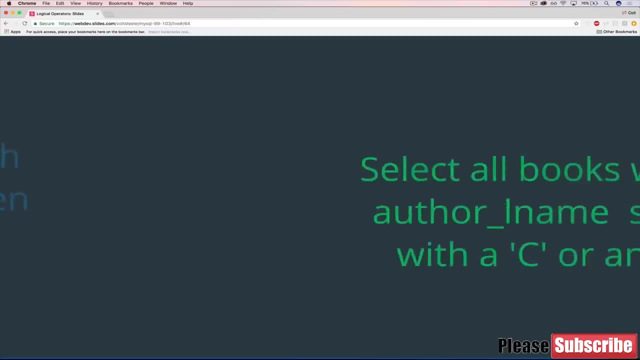 so if we didn't want to include 100 and 200, we could either do this or we would have to change this to be 101 and 199 or something. ok, so I'll leave it as 200. moving on. select all books where the author. 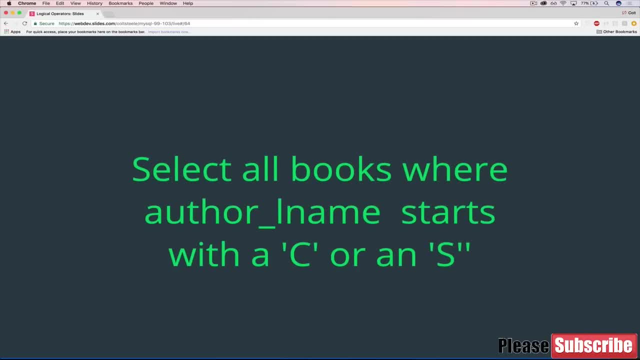 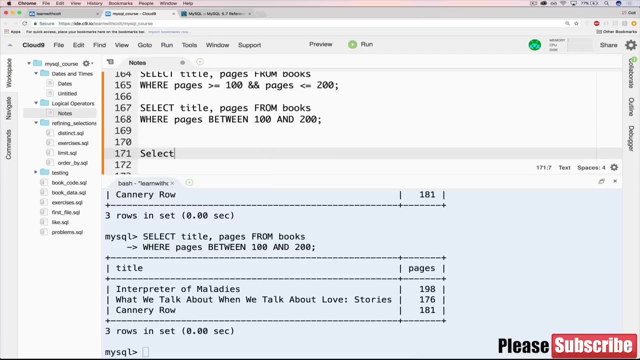 last name starts with a c or an s, so there's also a couple ways of doing this one. we'll start with the simplest one. so we want to select- and this time we'll do title and author lname from books and basically we want to- let's just type it out. 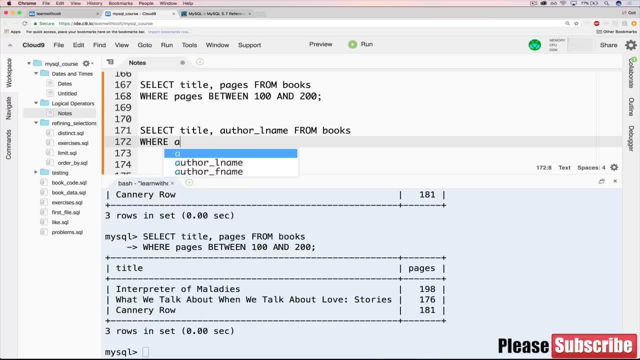 with the pseudocode or our english code, so where author lname starts with c or author lname starts with s, so those are not valid code. so how do we do this? there's a couple options. the first one is to just use like, if you're comfortable with that, instead of starts. 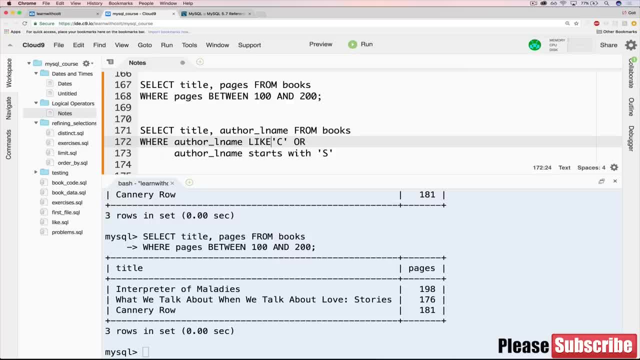 with c. we can just say where, author, lname like, and then we use the percent sign to force the c to be at the beginning of the string. so remember that this says string starts with c and then anything afterwards. so that's one way to say it starts. 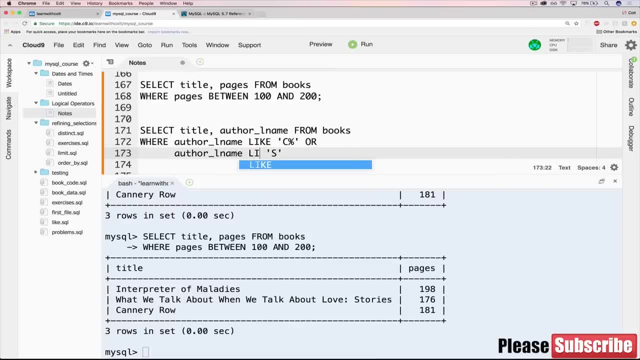 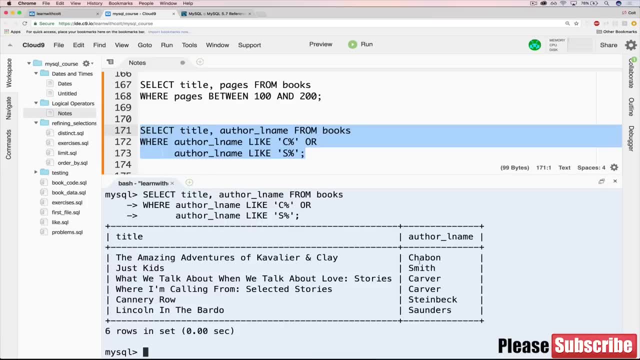 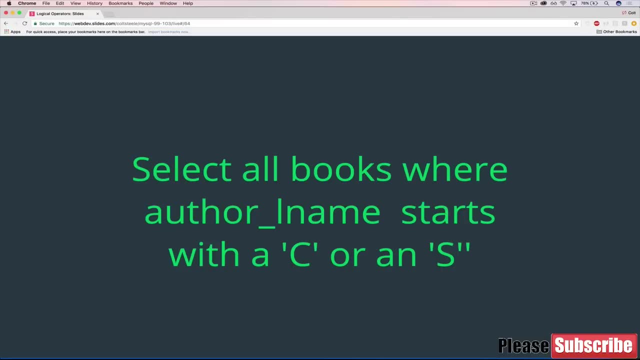 with a, c, and then we just do the same thing down here, like s, with the percent sign after that, and that should do it for us. so we get shaven. smith, carver, steinbeck, saunders- good collection of authors. however, there's another way, which is to use substring. 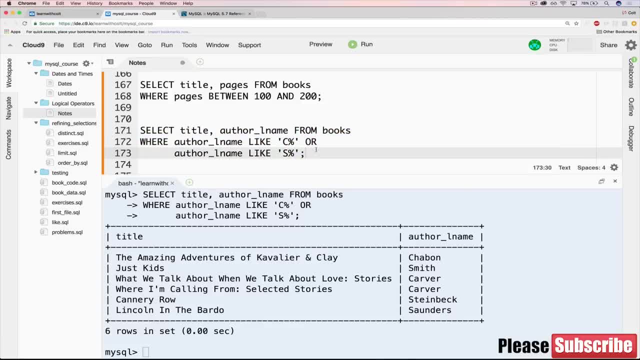 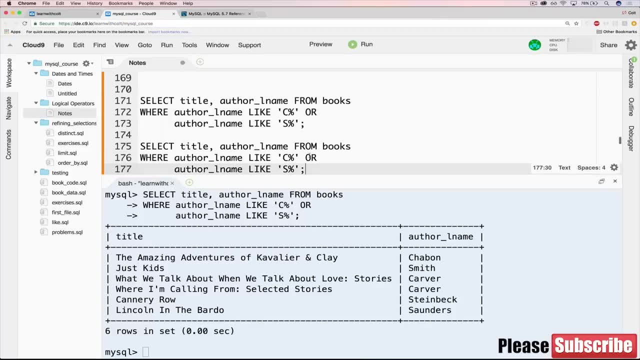 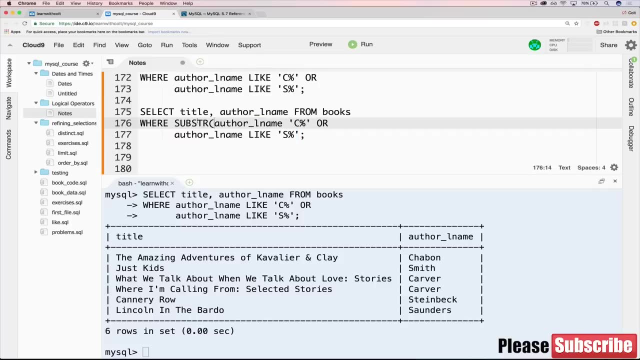 so if you remember substring- or maybe you remember me complaining about how there's also an abbreviated substr version- so we could use that, so we could say: we're author lname, substr of author lname, and we want one comma, one which will give us the first character. we want to check where that's equal to. 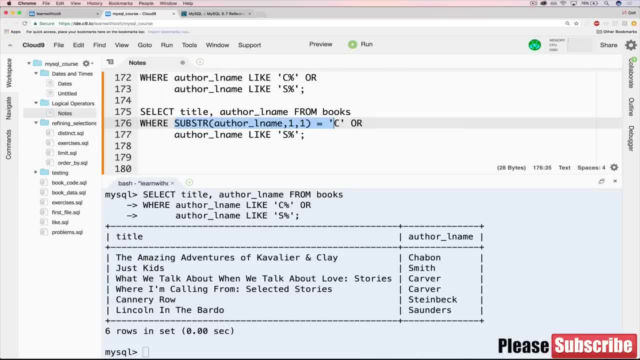 c, or, and i'll just duplicate this whole thing where it's equal to s. so we could do this and we get the same thing. but there's yet another way to clean this up, which is to then i'll just keep them all here so you can see them all. 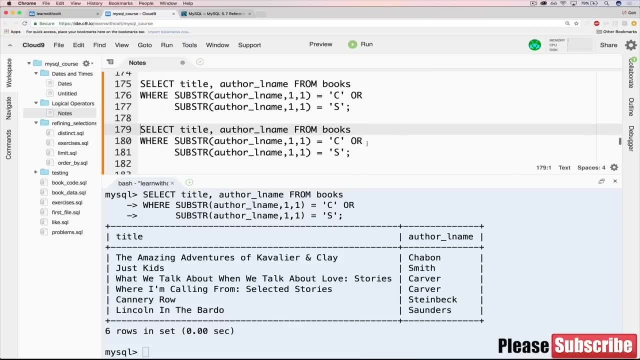 we could go, and because we're checking these two values, we could also use in c comma s, just like that, and get rid of the or. so now we're saying select title and author lname from books where the first character of author lname is in the set of c. 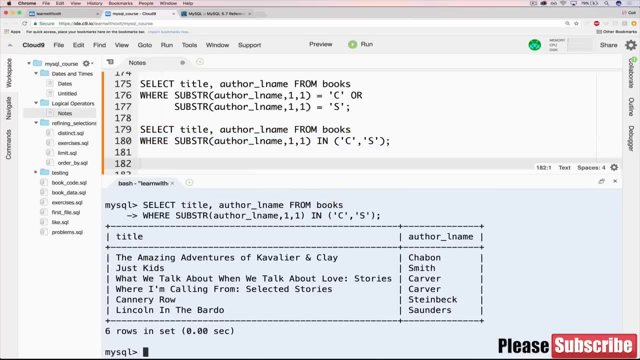 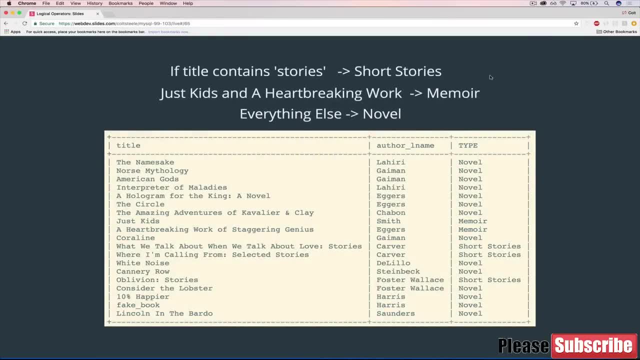 or s and we get the same result. so three different ways next up, moving on to case statements, so in this one i tried to throw you for a little bit of a curveball because, unlike the other case statements, we saw where we were just using greater than and less than. 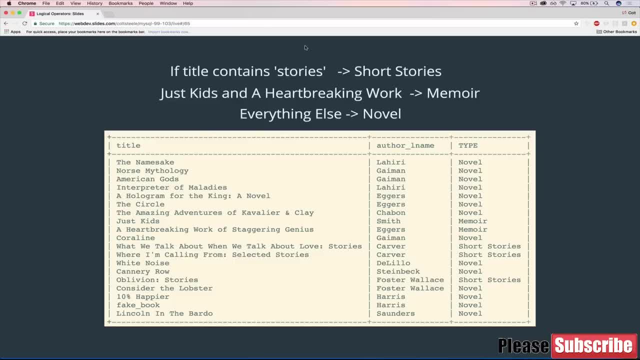 there's a couple things you're doing here, so we're just working with title, but you're seeing if title is like stories, and then you're seeing if it exactly equals just kids or a heartbreaking work of staggering genius. so let's start off with the basics: select. 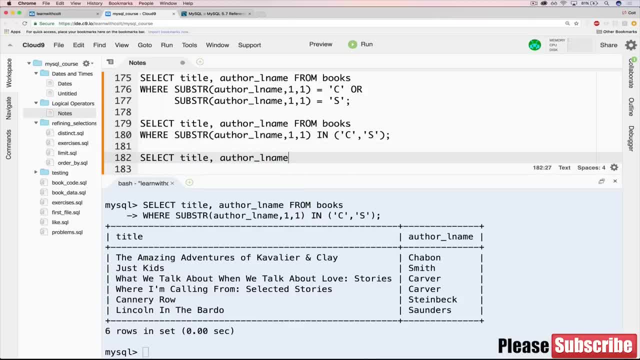 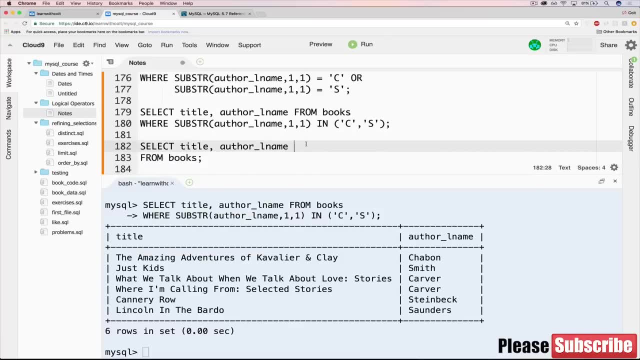 title and author lname, and we'll just do from books, just like that. and then we need our case statement syntax. so we're gonna have case and i like to just put my end right in there, as well as my as, and i called it type, which i don't actually think is a. 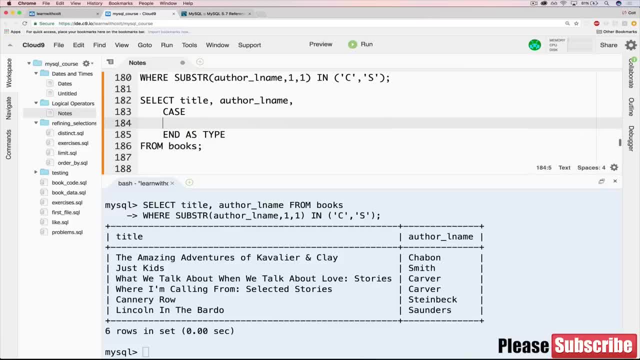 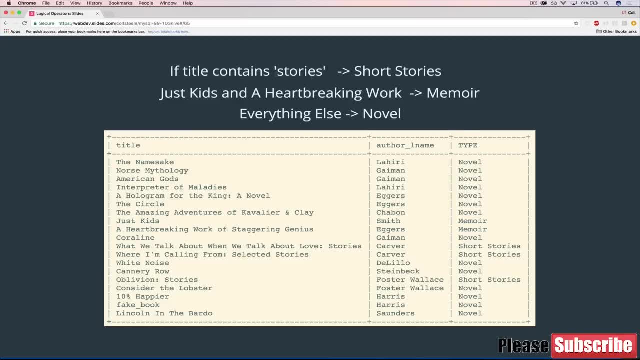 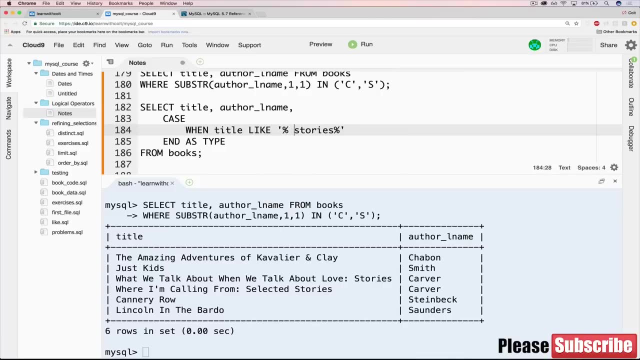 great name genre would be better. but inside of here we're gonna have our statements, so the first thing we're gonna do is figure out: okay, if title contains the word stories, anywhere type is short stories. so when title like, and how do we write or express the fact that it can contain? 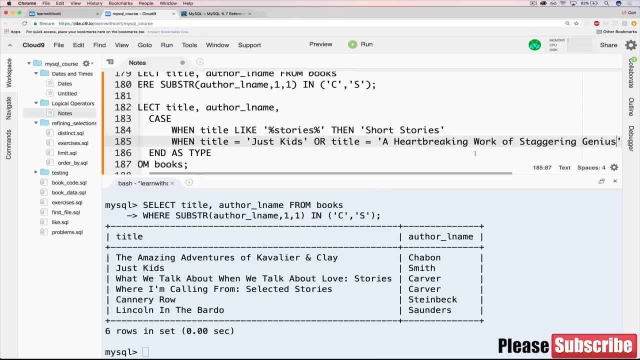 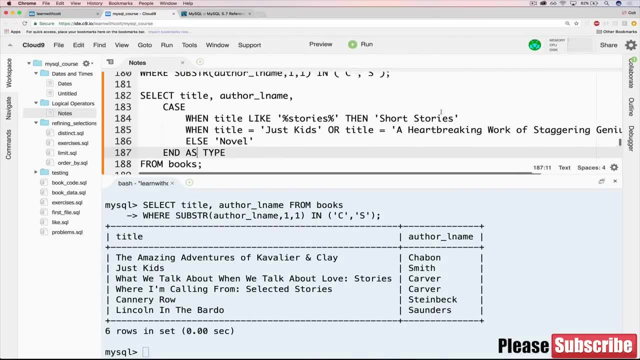 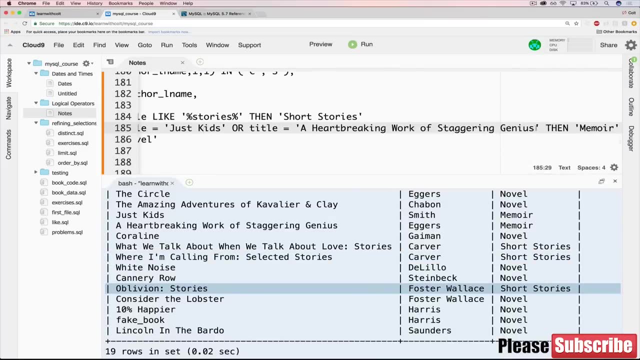 stories anywhere, not just at the beginning, but anywhere in there. well, we use parentheses, excuse me, percent sign. so this means that it contains a string stories with anything afterwards which technically we could have histories or something whoops, which maybe is not what we want, but we can leave it at that. you could put a space. 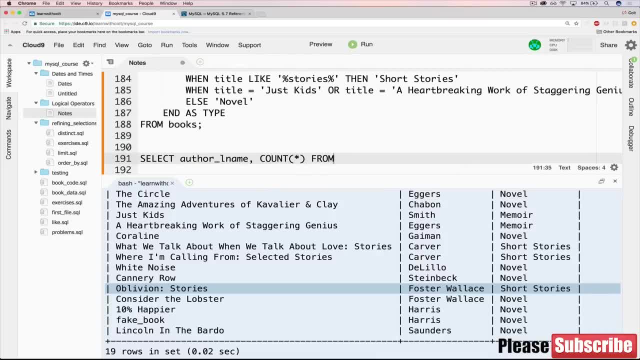 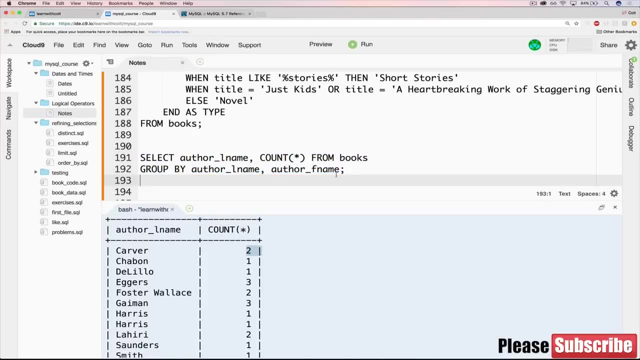 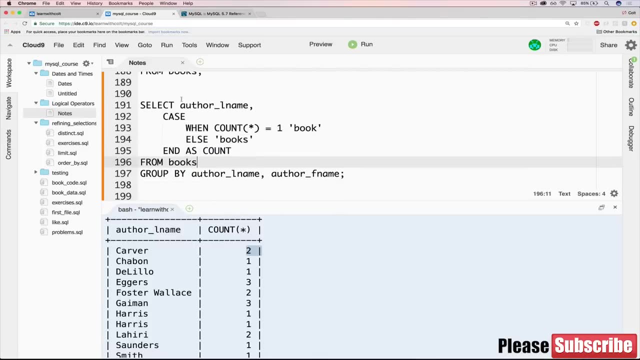 here or something to make sure that's just stories. but i'll keep it simple. with stories like this, then that's going to be short stories, as our type. okay, then we have another statement when title and when title is exactly just kids or a heartbreaking work, a staggering genius. 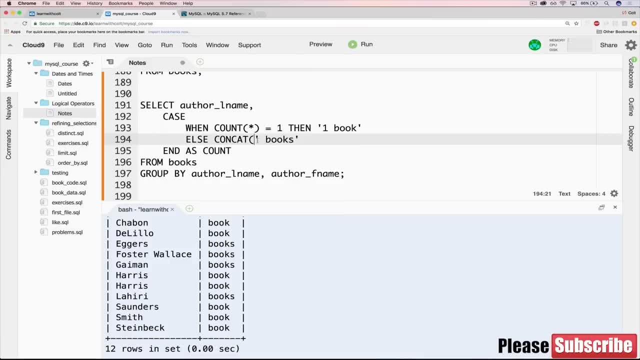 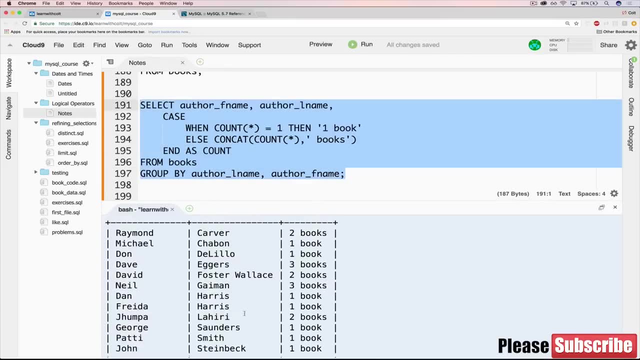 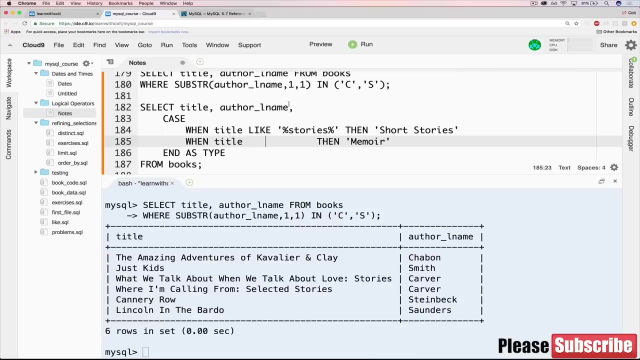 we should print out memoir. so let's leave that part blank and just add in then memoir. so then how do we fill this part in? it's pretty straight forward. it's gonna be a bit annoying. so how do we check if it's equal to just kids when title: 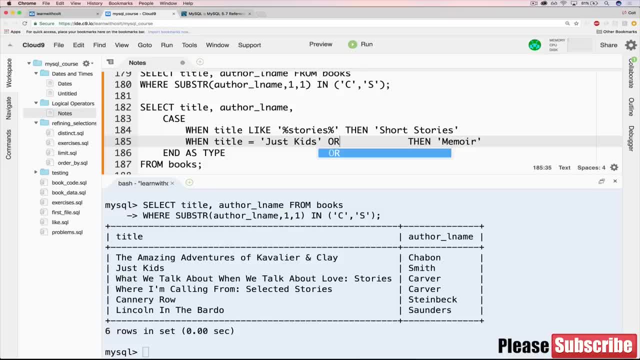 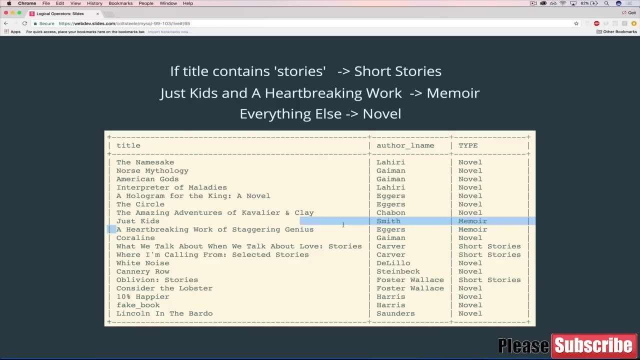 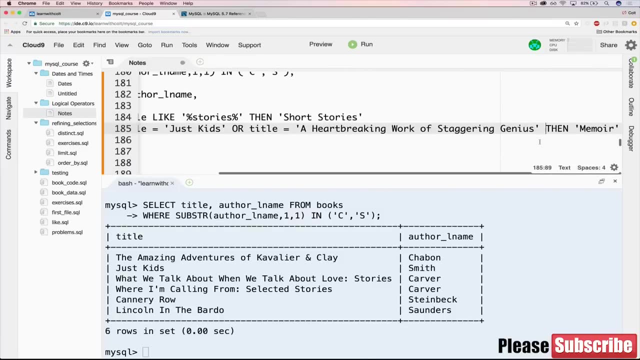 equals just kids, or when title equals- and this is gonna be very long so i'm gonna copy it. where are you just like that and i might shorten that. i definitely would shorten it. so maybe it would be better to use like or something and search for a particular part rather than the entire. 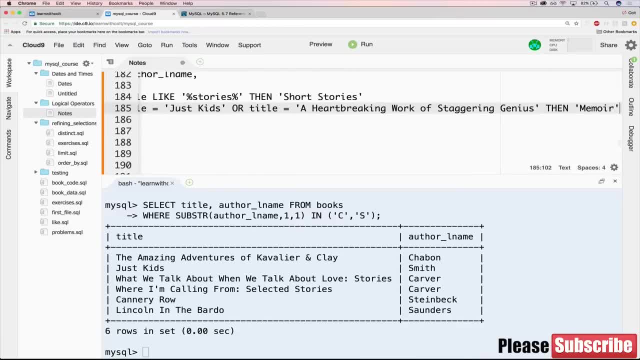 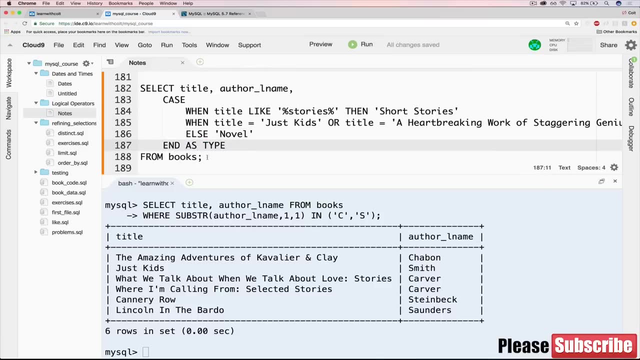 name- but that was a problem here- followed by our else, which is otherwise: everything is a novel. so that's where this comes in. else, novel, just like that. now let's double check. we don't have any extra commas, which i said i sometimes do. looks good, let's try it out. 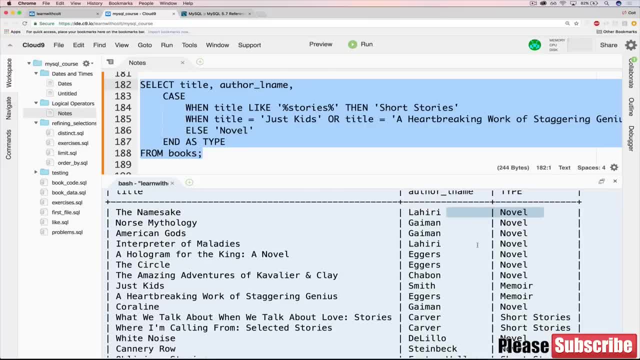 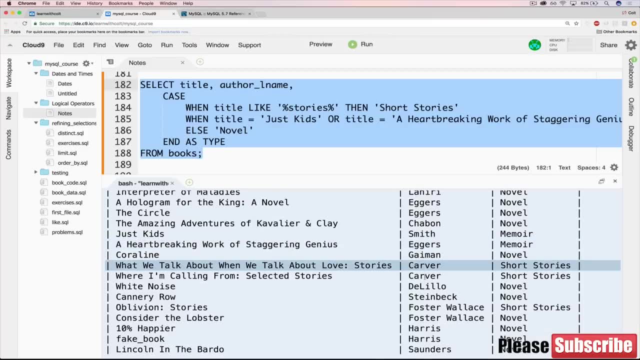 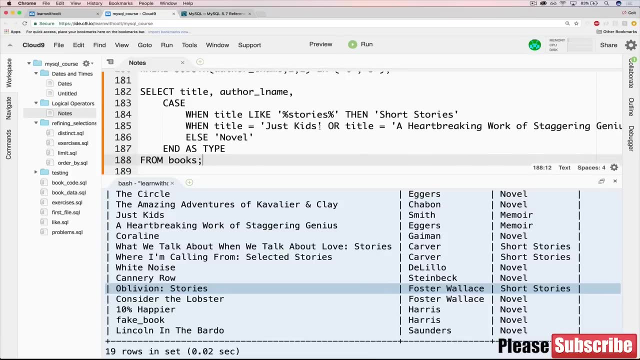 and we get all novels, except for just kids, and a heartbreaking work, a staggering genius. and then those are memoirs, and then we have two raymond carver collections with short stories and a david foster wallace collection. okay, so that's it, and of course you could clean this up. 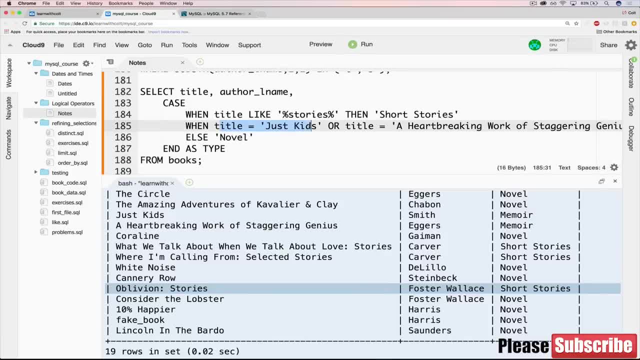 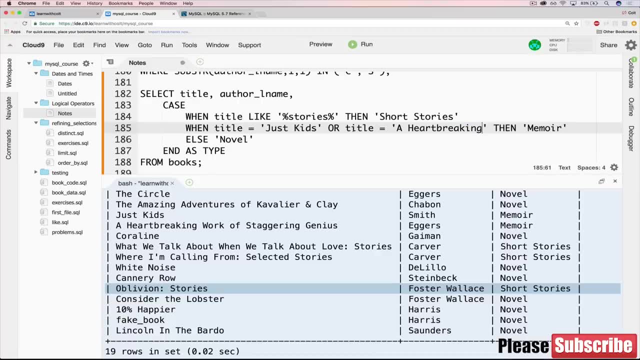 so you could have used in here title equals, so you could say: where title in just kids comma, heartbreaking work, a staggering genius. you could use like something like this or title like heartbreaking, although maybe we have multiple books with heartbreaking in the title, so i'm gonna leave that. 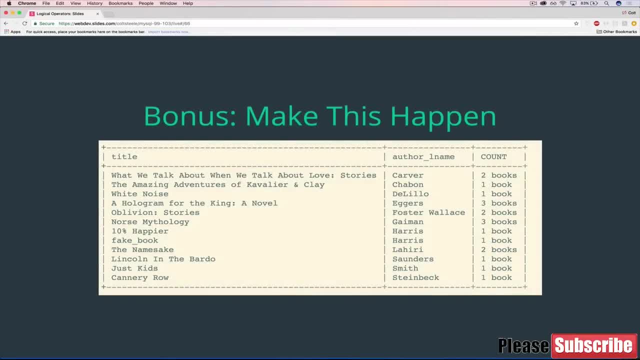 and move on to our final one: how do we make this happen? so again, what's happening? we're grouping things by author and we're counting how many books each author has written, but we're not just printing that out, we're printing it along with a space, and then 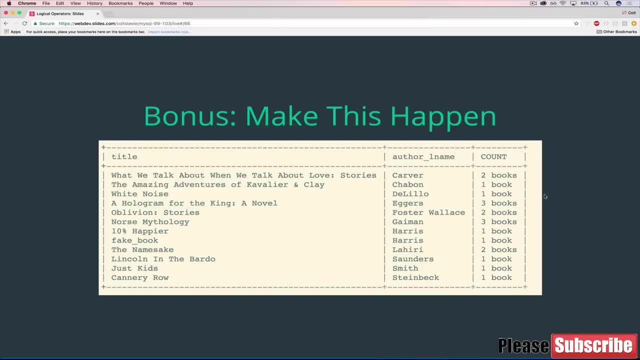 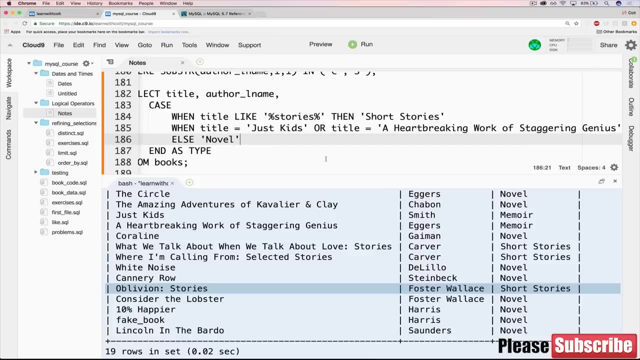 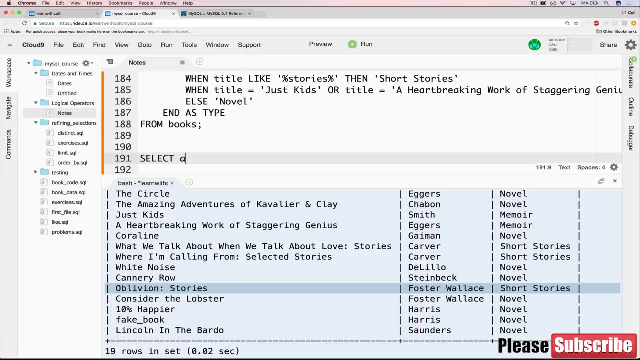 the correctly pluralized version of books. so we'll start by just printing out. we can ignore title, just do author last name and count without the books part. so that should be review of group by and count. so we'll select author, l name, comma, count star from books. 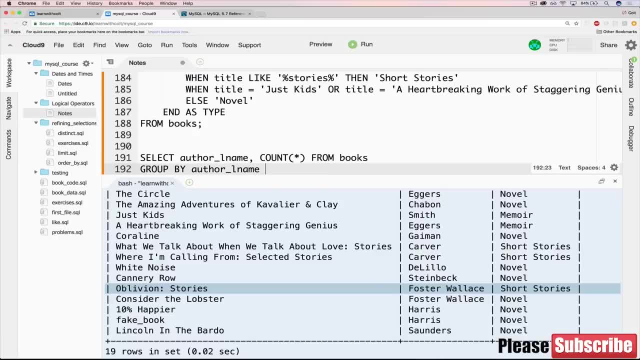 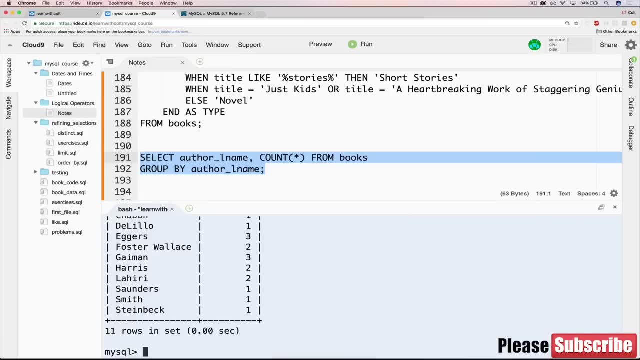 group by and we need to group by author l name. so if we do this, oops, you'll see, we end up with: carver has two books, eggers has three books, and so on. we do have that problem with harris having two books, so we need to make this more specific. 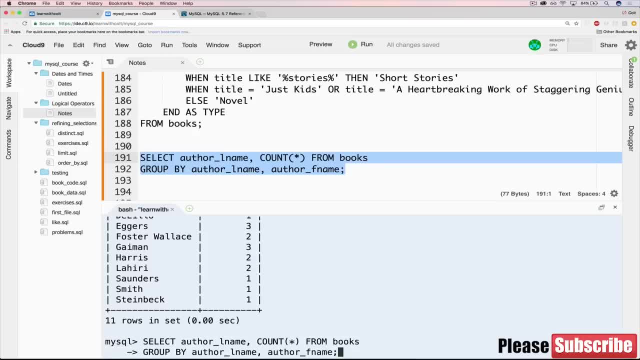 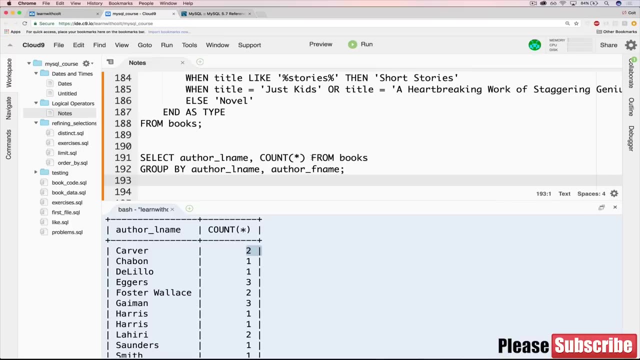 where we also group by author first name, and now we have two different harrises. perfect. so now, how do we, instead of just printing count like this, how do we add in that variable the changeable suffix book or books that uses the case statement? so i'm gonna make some space here. 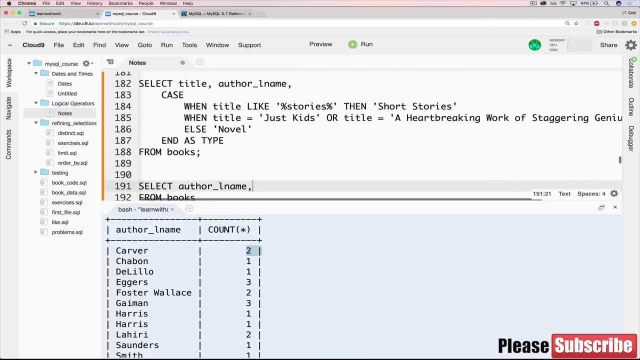 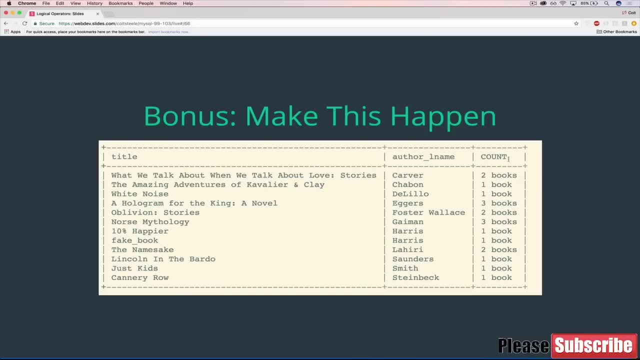 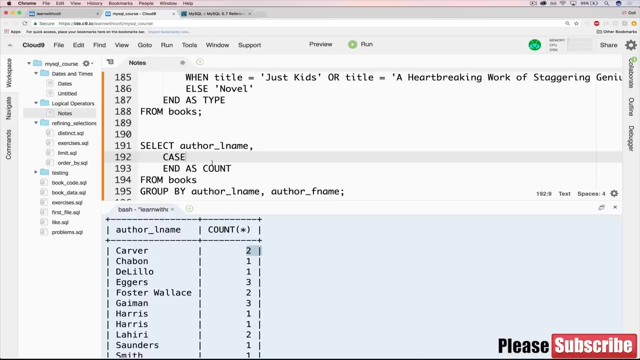 and rather than just printing the count, we're going to add, in our case, end, and if you look at how i printed it, i just called it count, so end as count. then what is the logic we're actually trying to do? well, we're trying to figure out. 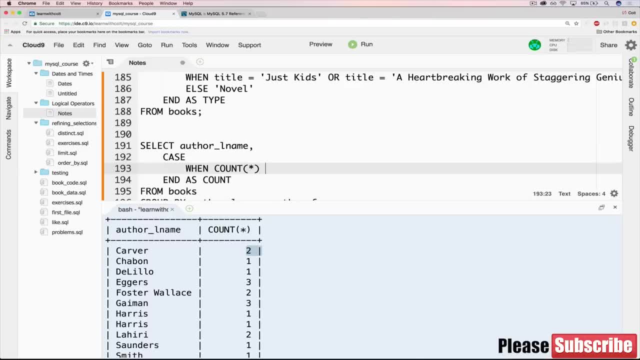 when the number of books count star is equal to one. let's say: then we want to do something, let's just say singular book. this isn't the right answer, otherwise we'll do books okay. so the logic is not going down the right page. we're grouping things. 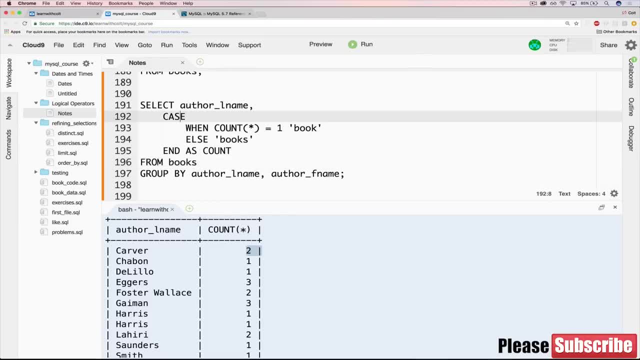 by author. then we're having a case statement that says when the total count of the number of books that author has written is equal to one, then count is book. and before i forget, we are missing our thens. so when count equals one, then book. that's very important. 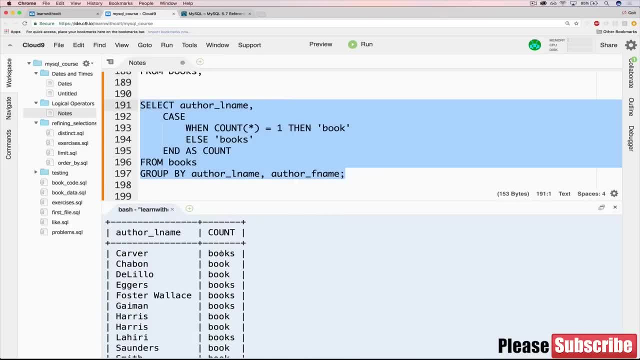 now, if we paste it, okay, so we get: carver has books, eggers has books, but each harris has book. so we're close. but how do we get the number in there? and we need to use concat. hopefully you guessed that, so we're going to concat. 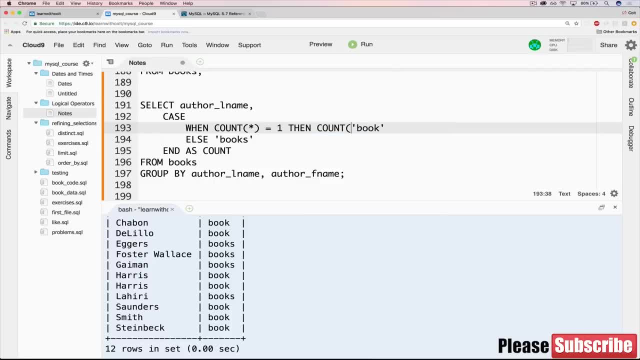 basically, we want to take the number which is going to be count, and we want to concatenate it with space book. now, if we want to shorten this, we could just hard code this as one book, right, because when count is equal to one, then it's always going to be one book. 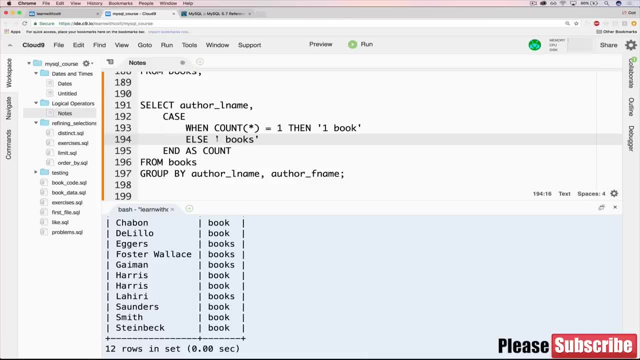 this is the one where we have multiple books. we need to add in the number because it could be two books, it could be ten books. so we'll concat the two pieces which are going to be count star comma, and i know this looks like a lot here. 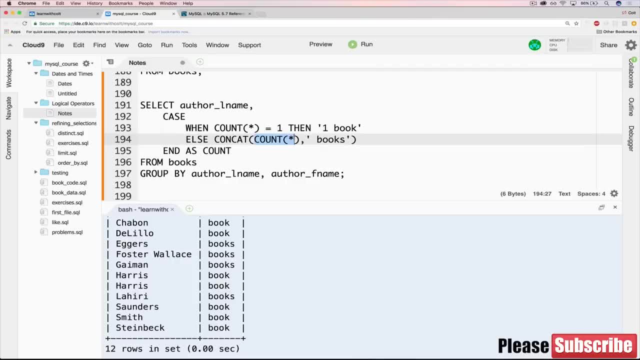 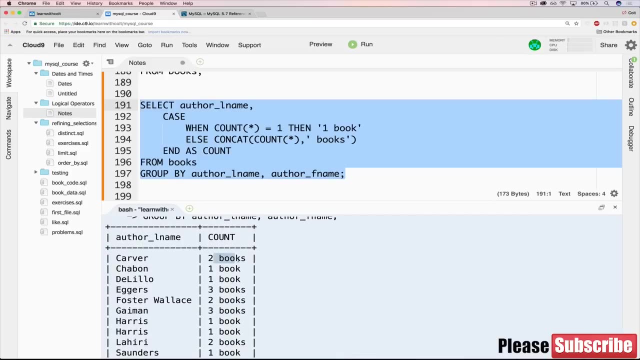 so let's step through it, concatenate the count with space books. so two books, three books, and that should do it. let's double check. here we go. carver has two books, shaven has one book, harris has one book, lahiri has two books. the only other improvement, i guess, to suggest. 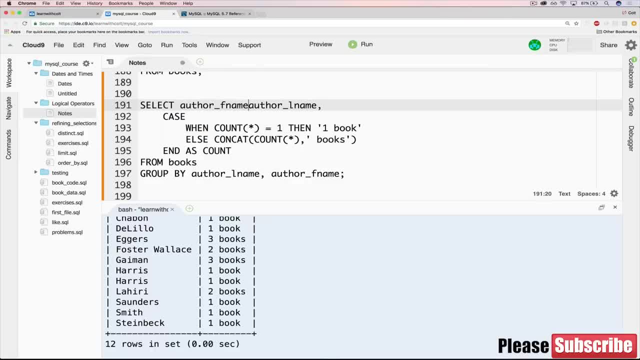 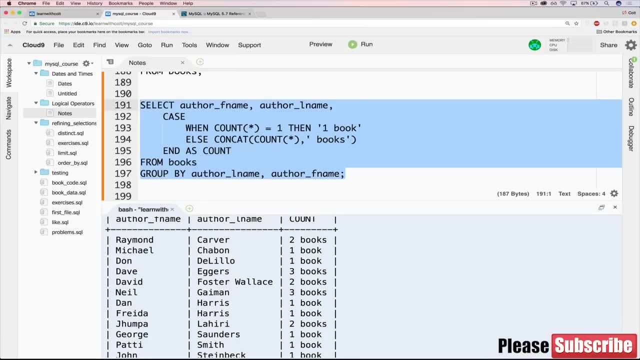 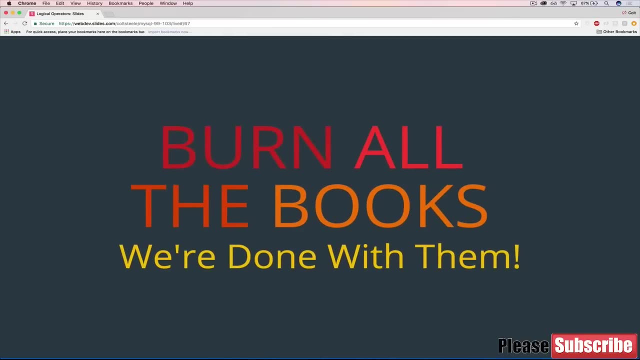 would be to also put author first name, just to make it a little clearer. in the case of harris, we now can see: dan harris has one book and frida harris has one book. jhumpa lahiri has two books. alright, so we got a bit there. 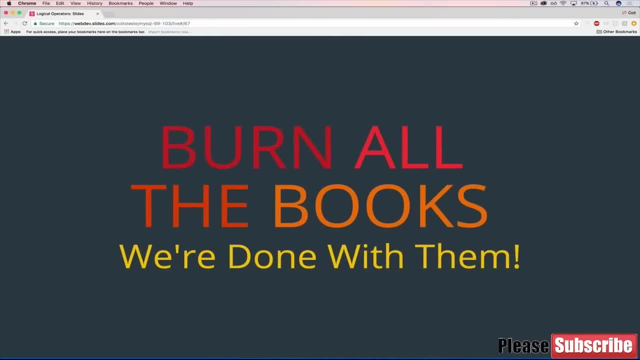 hopefully you made it through time to move on. we can burn that part of us that's attached to the books. we are done. we're moving on to bigger, more exciting things. i highly recommend that you, if you're at your computer, get up and take a break. 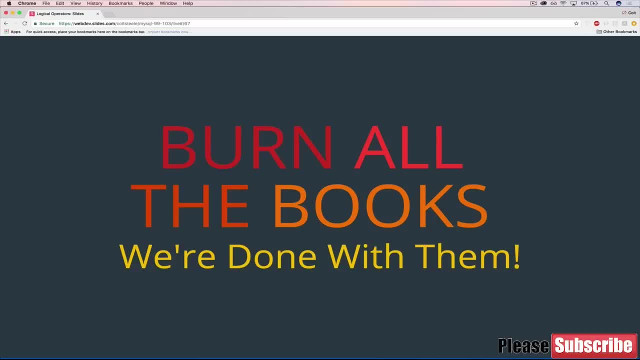 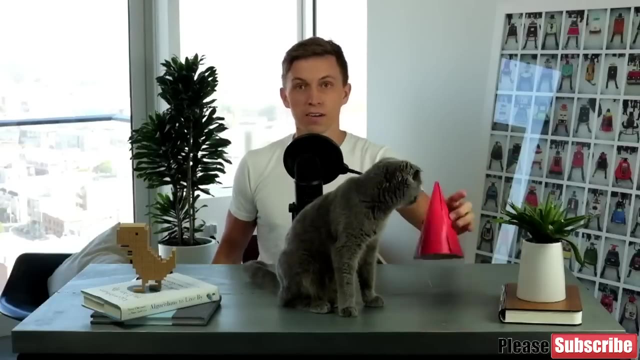 because joins are a big section, very important stuff coming up next, but a bit dense. so go for a walk if you'd like or do whatever you need to do to get prepared to focus on joins. so this section is a big one, really exciting stuff. i mean, exciting is relative. 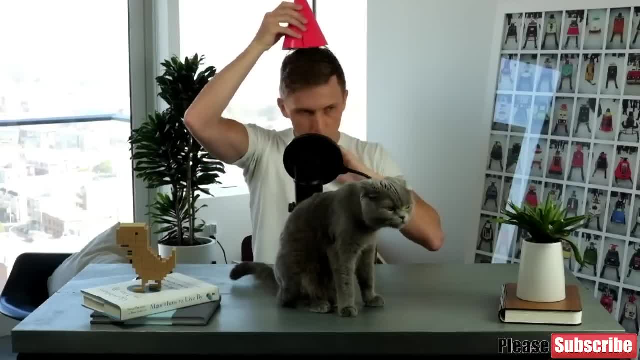 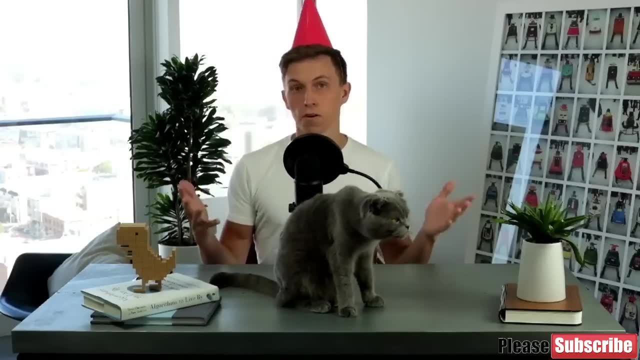 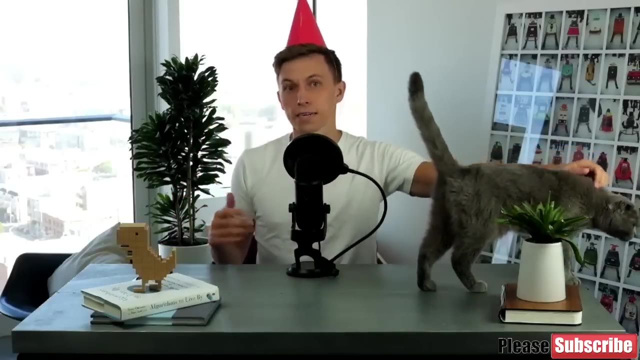 we are talking about databases, but i do have a party hat here to celebrate, yeah. so let's see what are we talking about here. this course has been so far all about data in basically one table at a time, kind of self contained basic data- nothing all that exciting. 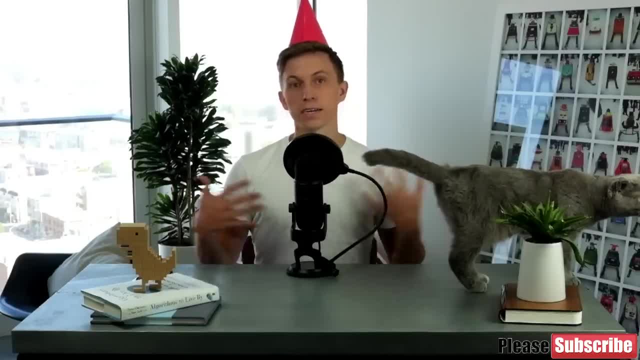 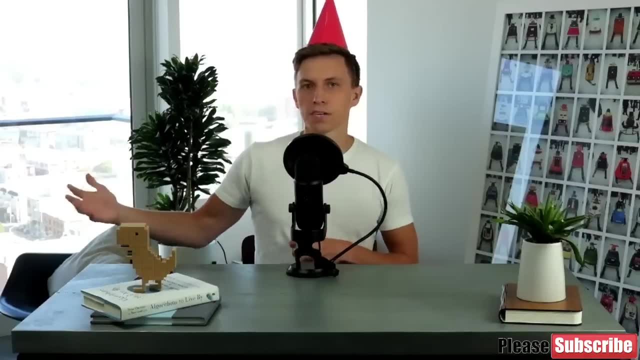 and nothing very complex, no data that is related. but of course, in the real world, all of our data, or almost all of it, is related. we don't have books on a website without also having things like reviews and customers and i don't know, shopping carts we don't have. 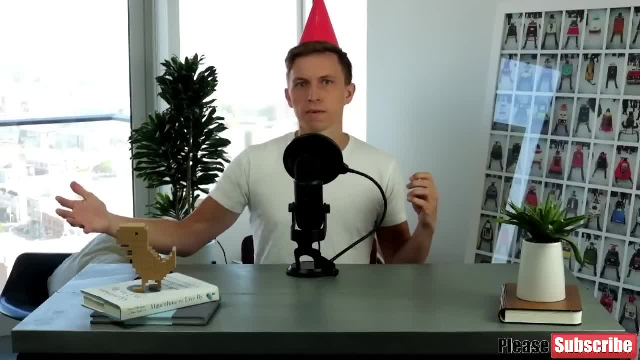 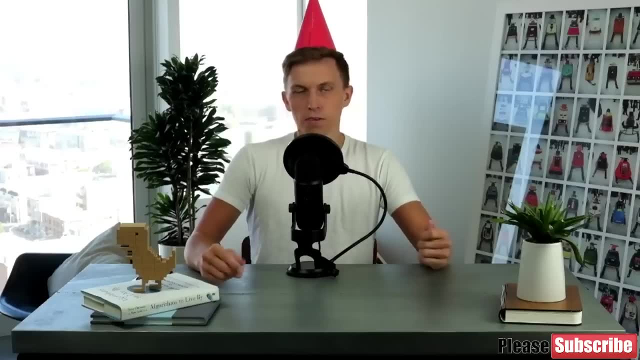 cars on their own. we might have cars in our database, but then we might have salesmen and dealerships and all the other things that go along with it or like on instagram. you don't have just photos. we have users, photos, comments, tags, likes, followings. 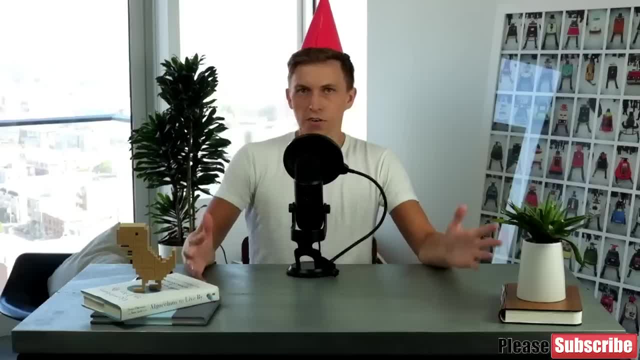 relationships, all this stuff that's related. so this is a turning point where we well, one of the turning points where we start to work with multiple tables that are connected. so we're going to talk about how data is related and then how to implement those relations using multiple tables. 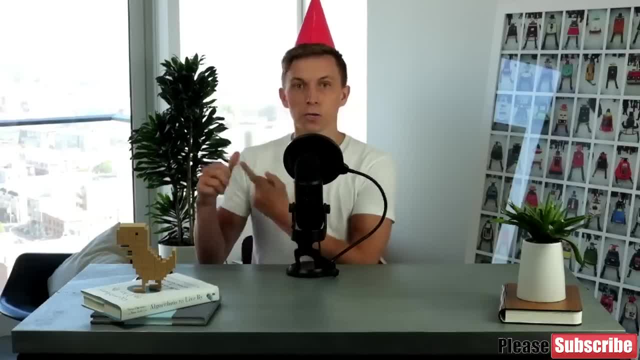 and some of the buzz words, some of the big things we're talking about here are joins, foreign keys and primary keys, which we've kind of seen before. one to one, one to many, many, to many relationships, lots of stuff. but, like i said, this is the first of a couple sections. 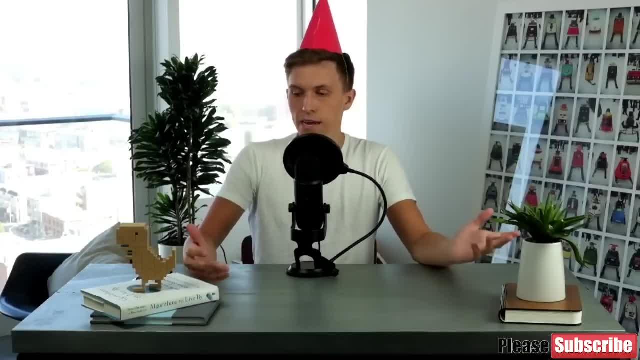 on related data. and the other thing that you may want to celebrate is that we are done with our books, done with the books data. you can totally go burn the books if you'd like, throw them off a cliff. we're done with that. we're moving on to bigger and better things. 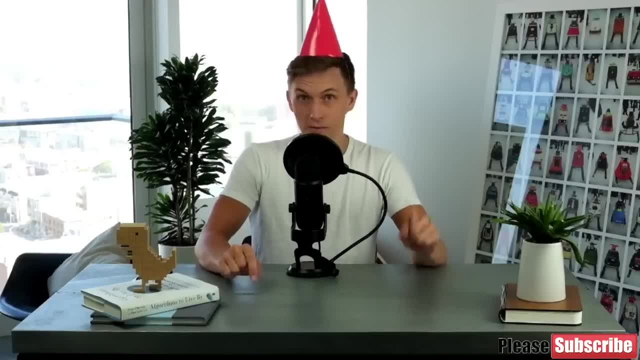 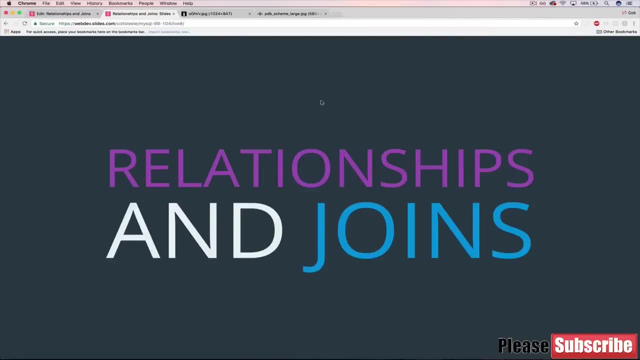 inching closer to our instagram data at the end of the course. okay, have fun and don't forget your party hat, because i didn't. yeah, okay, welcome back to the course. this is a really important section, not to scare you too much, but really fundamental to how sql and mysql are used in the real world. 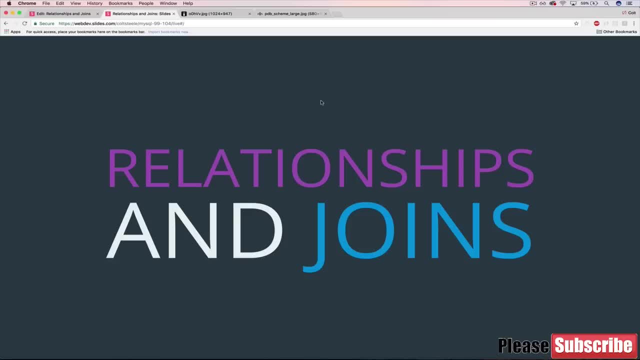 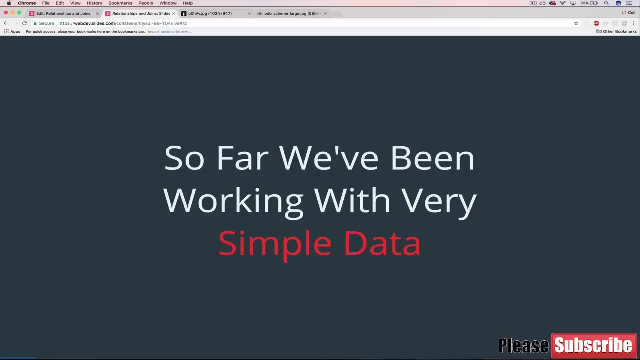 so this is a section all about relationships and also something called joins, which we'll get to in the second part of this section. so let's focus on the relationships part first. so far in this course we've been working with very simple data, things like books or users. 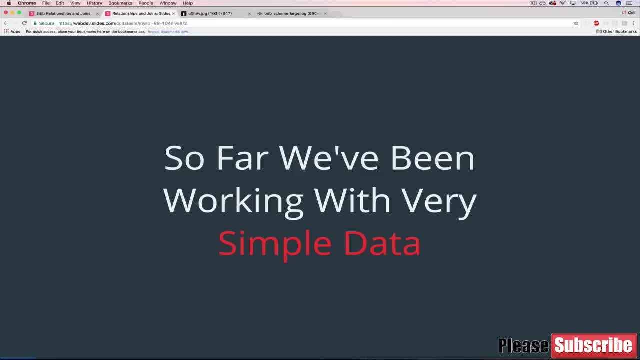 where we only have a couple of columns per table, and that's been by design. we need that simplicity in order to focus on what's important, to isolate the different features that we're talking about, whether it's functions or logical operators. it's much easier to teach those when we don't have. 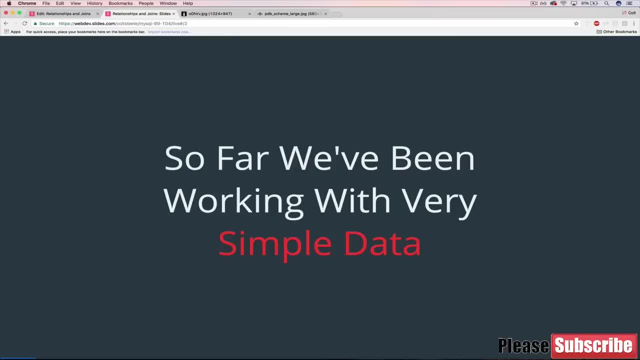 20 different tables to worry about and we can just basically drill down into one table and focus on that. but that's typically not how the real world works, where, yeah, we might have a users table, but it's a website that really can just get by on having users. 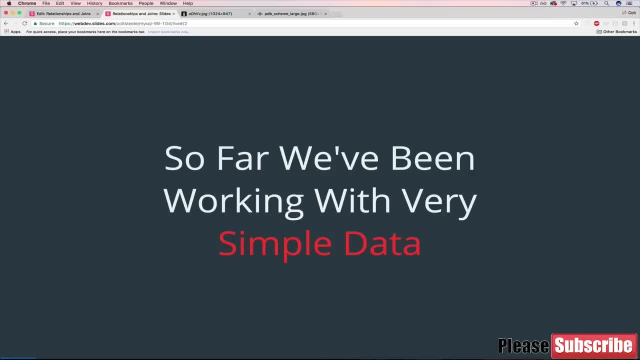 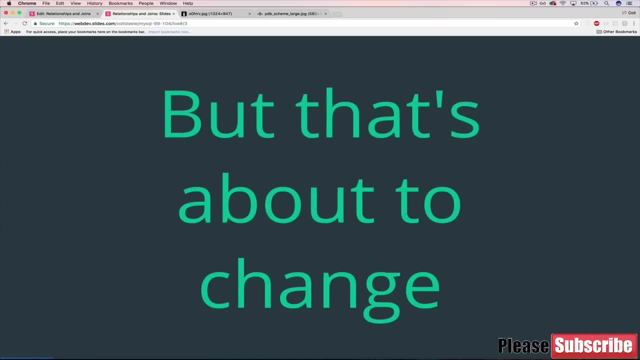 unless it's featureless. there's plenty of other things that need to go along with users, whether it's comments or likes, or tweets, or posts or photos or any sort of order transaction. there are all these different things that we could have alongside users, so we've been working with simple data. 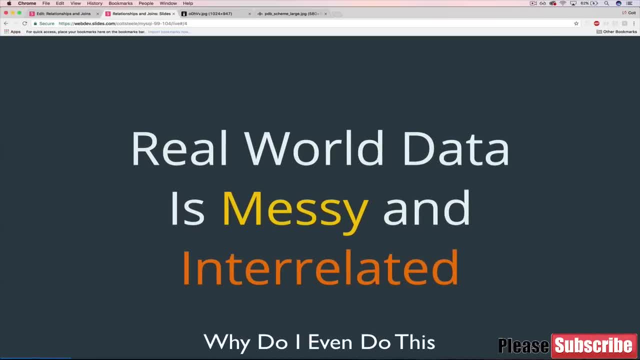 but that's about to change. real world data, unlike what we've been working with specifically and interrelated, there's a lot of connections between data, so some of those things I talked about with, let's say, users, if we're working with just a simple blog site, 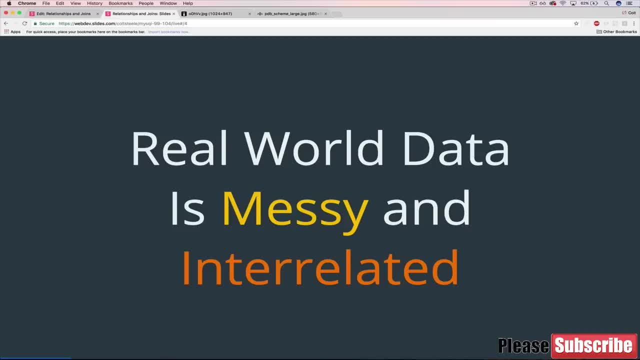 so nothing like a Facebook or a complex social network, just a simple blog. we still need to have user data, we need to have information about posts, blog posts. we also need to somehow keep track of comments and then tags, and that can get pretty complicated already, not to mention things like advertising. 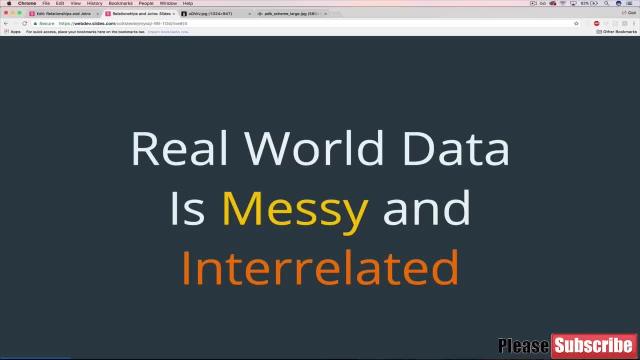 and how ads are related to users and what users are clicking on and not clicking on. there's so much data that just from a simple blog site- something that may not seem that complex- there's so much stuff that we could store, so we're going to focus on. 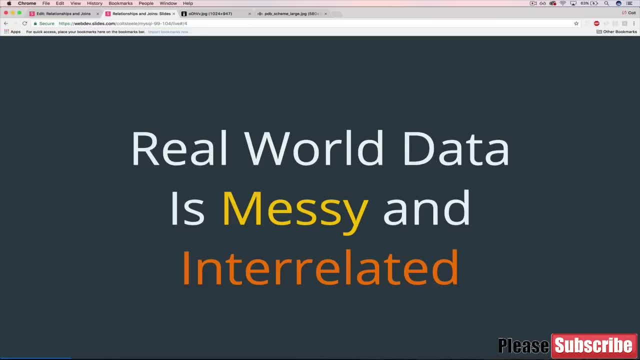 how we work with interconnected data in the next couple of sections. so we're no longer focusing on one table, we're going to see how do we work with two tables, or three or four that are related, so not just tables that exist independently, but tables that reference one another. 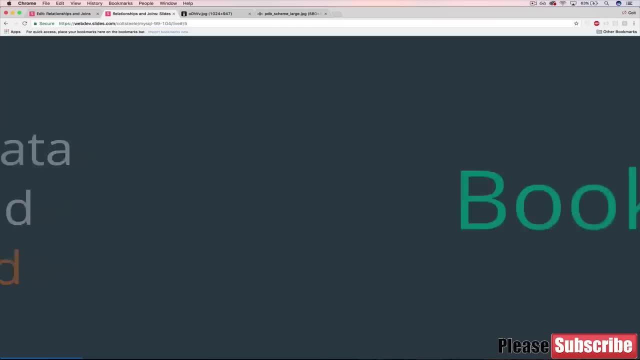 and are interconnected. so let's get going, and the first thing that I want to do is go back to our books data. so remember our books table. don't worry, we're done with it. we're not going to be typing any books code, but on its own it was really simple. 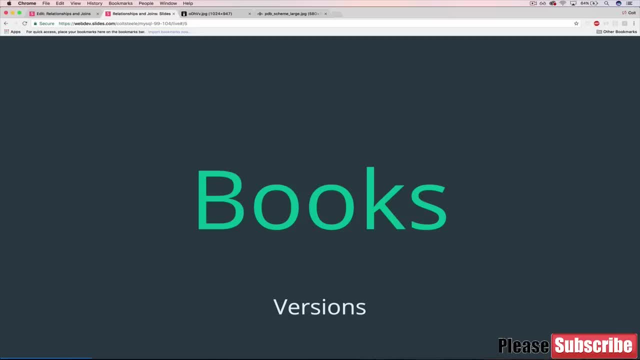 we had a books table with author, first name and last name, a book title, a release year, a page count and a stock inventory, I believe a stock quantity, and I think that was it. so again, on its own that just represents a single book, but if we were running a sort of 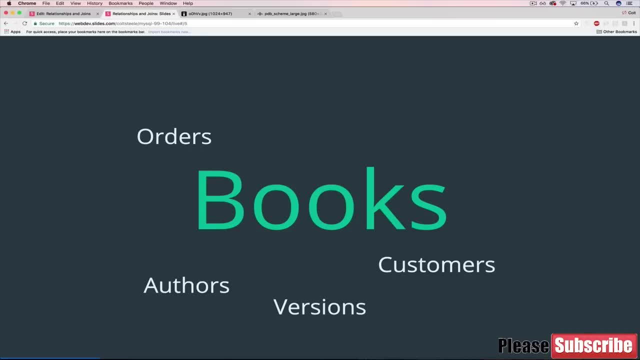 book site where we sold books. at a minimum, we would need to keep track of things like versions. so we didn't even talk about this, but there's often multiple versions of a single book if you go on Amazon and you look at a book, let's say Harry Potter. 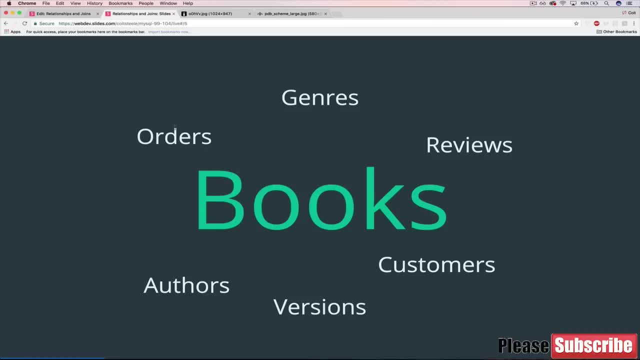 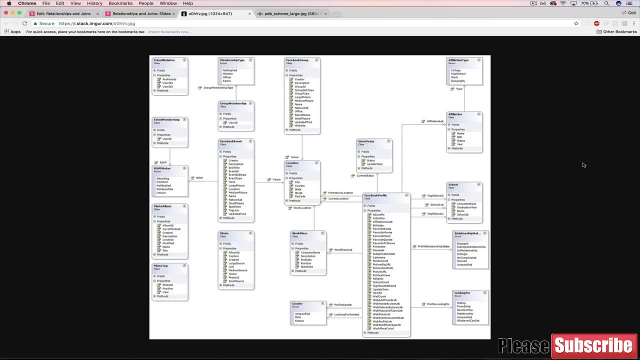 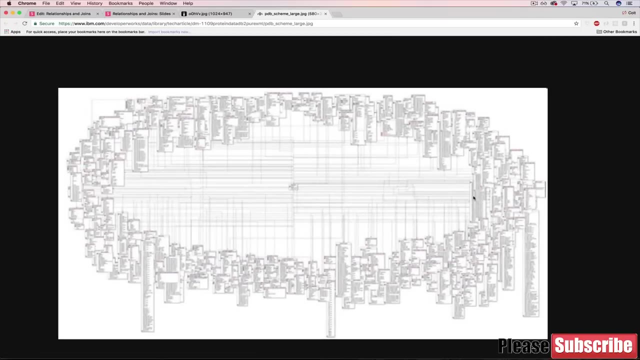 the second book, Chamber of Secrets. well, there's going to be the initial British release, the UK version as a hardcover, and then there's a paperback, and then there's the American version, and then there's a paperback that came out relatively recently. looks pretty cool, that has these giant illustrations. 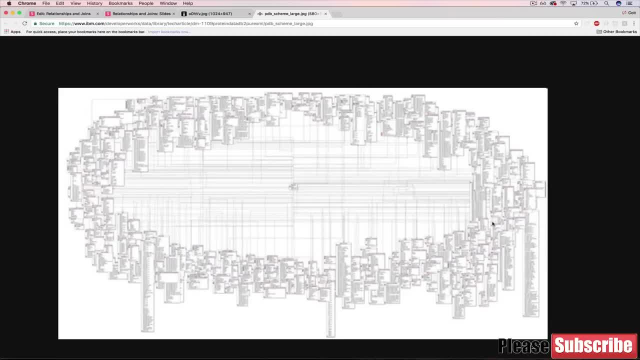 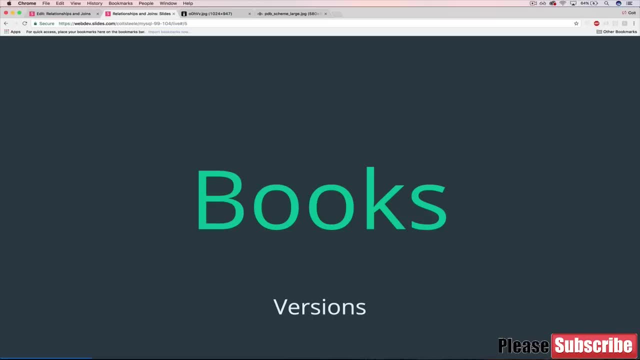 it's the same title. how do you keep track of that? is that a different table or do you just make a separate book for every one of those? but if you do that, then how do you make sure that they're connected? because when I go on Amazon, 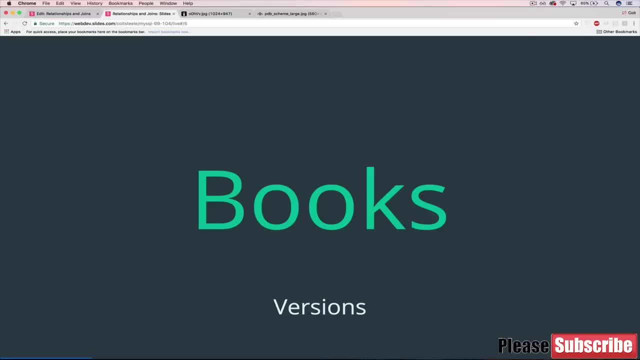 and I look at the hardcover. it also will show me below. some people also buy paperback version or it's also available in I don't know 25-40 different languages. so there's all sorts of things to worry about just with versions. but then we have authors. 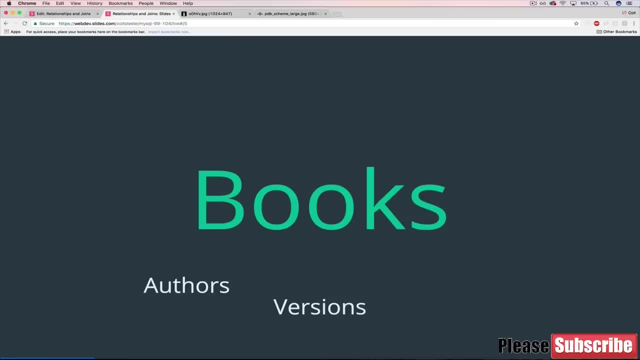 well, that might seem straight forward. we have an author, first name and last name, two columns on our books table, but that's not sufficient when we have multiple authors. so some books, a lot of books, have multiple authors. what about if it's a research paper that we're selling? 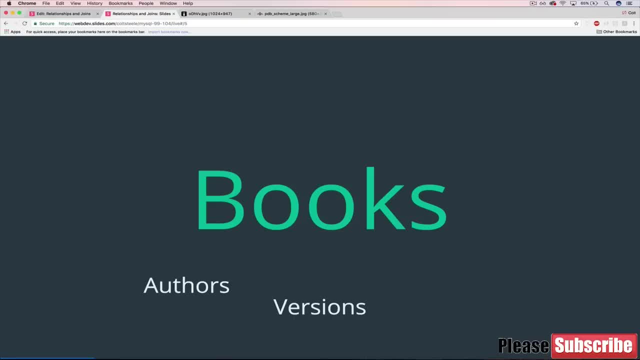 or a journal that has dozens of authors potentially, so there's a lot of things to keep track of there that we can't really do right now. if we have one author in our columns, then a whole big thing is customers. if we're doing a book shop online, 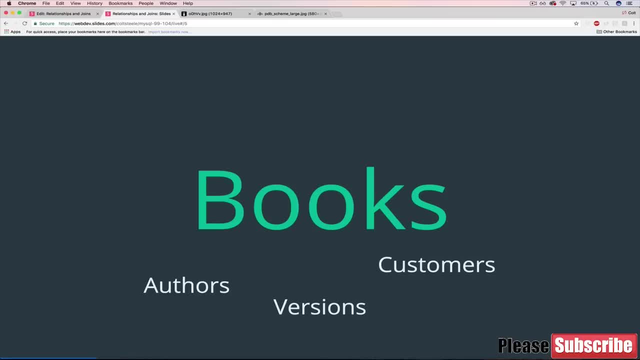 books on their own is great, but we also need ways to keep track of users, or customers, is what I'm calling them in this case. so customers on their own also can't do that much, but we might keep track of their email login information. of course, we wouldn't just store their password directly. 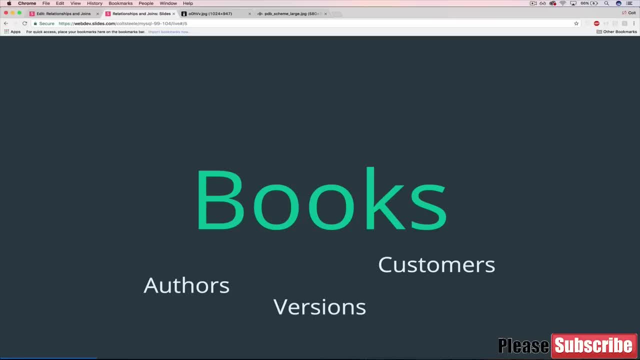 but for simplicity's sake, let's say we're keeping track of password and email so that they can log in. and then there's a whole bunch of other things: orders. so if customers want to order books, how do we store that? we need to create a new order. 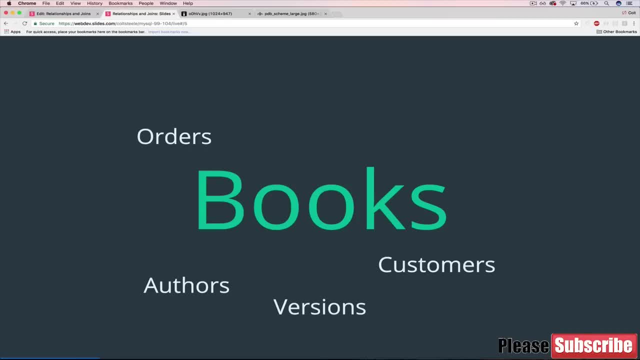 and it needs to be associated with the customer who created it. it needs to have address information. maybe it needs to have the contents of the order. are there books? one book? how do we support that? how do we handle that? what about if we're working with dates and times? 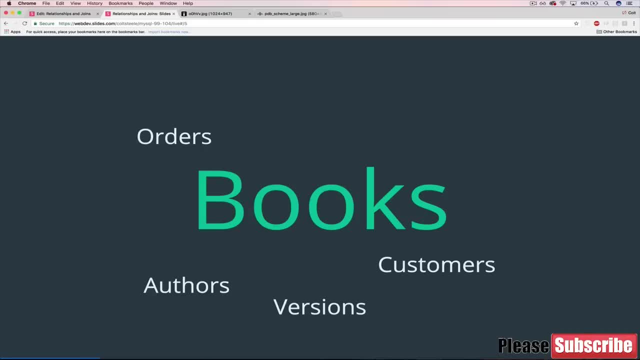 and we need to keep track of when a return period expires. so we need to have an order date and then keep track of 30 days or 60 days after that or whatever it is. then we also need to store or somehow keep track of the transaction information. 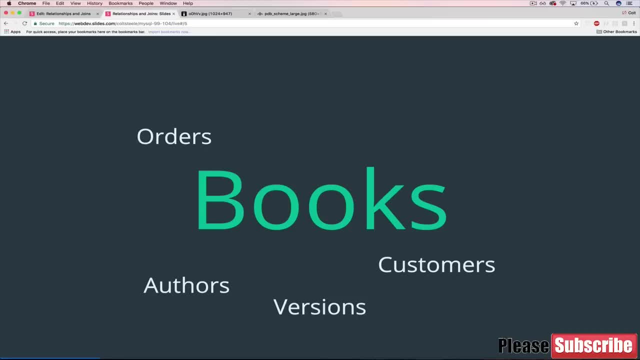 addresses for billing address, not only shipping address, the type of shipping, the billing information. there's so much to store. and then a whole other thing is reviews. so if we go on Amazon or pretty much any book site, any book that you look at will have dozens or hundreds. 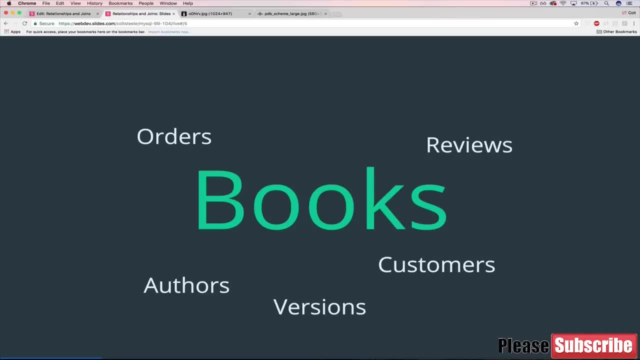 of reviews. so we've got reviews there, ratings, the number of stars, but then also a title for the review and then a caption and then the actual content of the review, which may be 10 characters. I hate this book, however many characters that is, or it could be a giant paragraph. 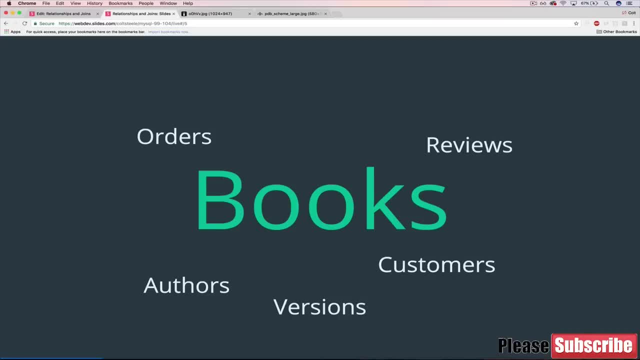 someone's love letter that they're writing to a book. so how do we account for all of that? and then the last thing that we'll talk about are genres. so you may think that we could just get away with storing this in a book, which we absolutely could. 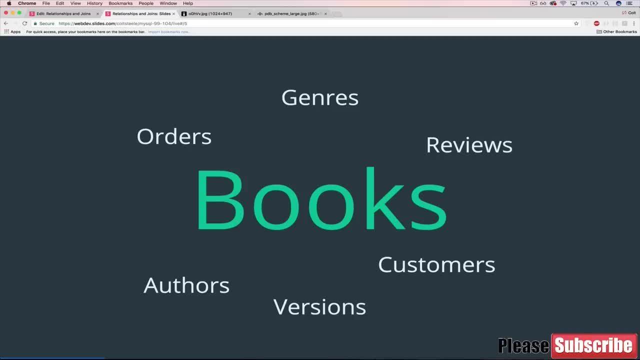 we could just have one genre, but many books don't cleanly fit into one genre. you might have a vampire novel that's also historical fiction because it's set in Victorian period England. or we might have a sci-fi book that has elements of fantasy, or who knows? 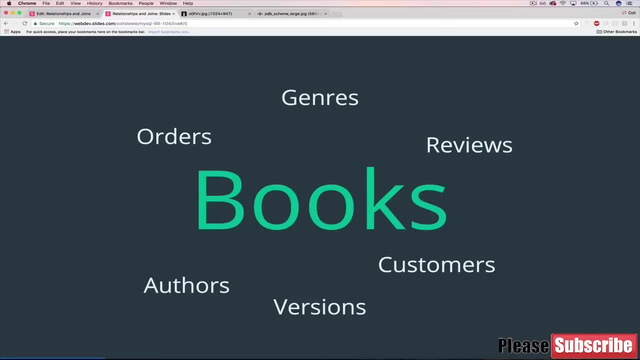 you can have all sorts of cross-pollinated genres, so only assigning one genre might not be that useful. we may want to have a bunch more, and in fact on Amazon you can see that we'll have two or three different genres or different tags associated with them. 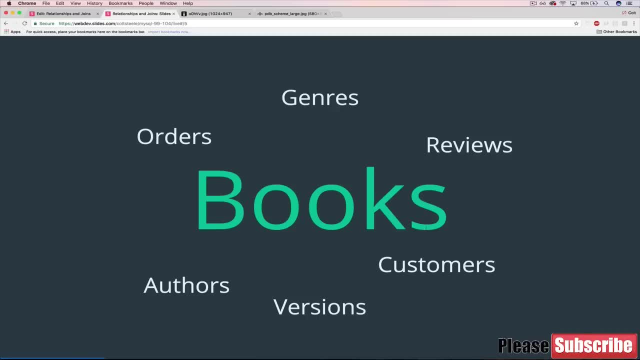 so what I'm trying to show you here is that we were working with books on their own, but in a typical app or typical website that has to do with books- a bookstore in our case- there's a lot more that goes along with books to make anything functional. 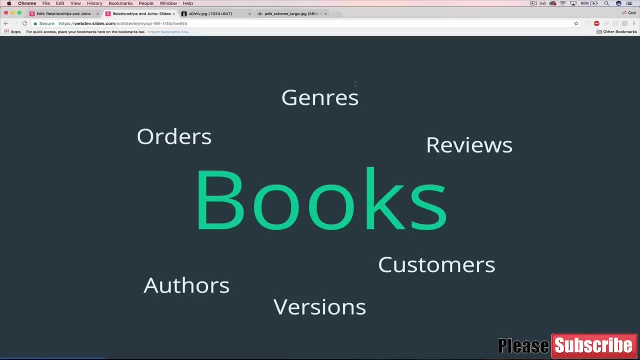 to store any important information, and this is, I don't know, maybe half of the tables that you would need to get away with, kind of the MVP or the bare minimum. there's still many other things, something like orders, for instance, might actually need to be split. 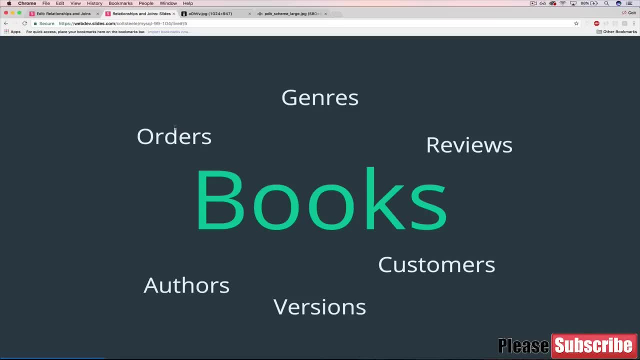 into a couple of tables. we might need to have an address section or an address table. we might need to then have a separate billing table. we might need to have shipping. there could be all different tables that we could split it up into. so this isn't to say this is the end-all, be-all. 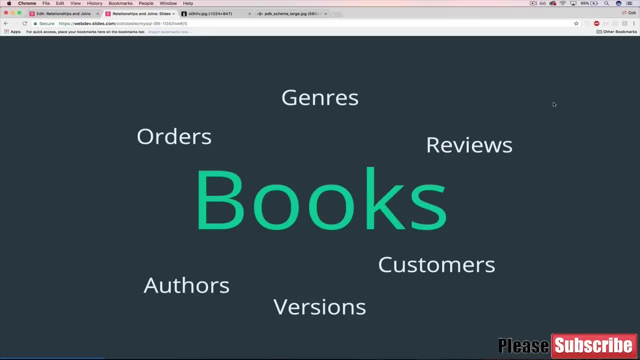 this is just that there's a couple of other tables that we need to consider at the bare minimum. okay, so we'll stop here. in the next video, we're going to identify some of the different types of relationships between data at a high level. what are the different types? 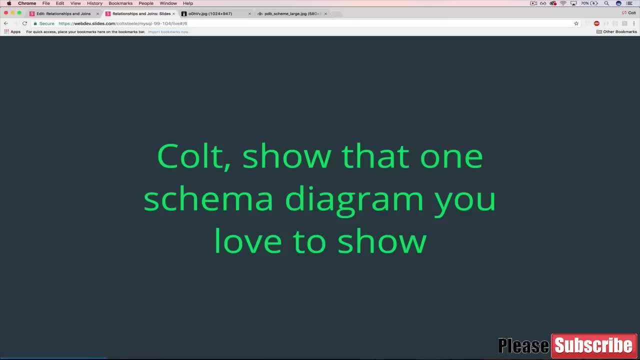 of associations, and I'm back. I totally forgot to show you this, even though I wrote a note to myself. I totally skipped this, so I'm back. after recording this, adding this to the end, I want to show the schema diagram that I really think highlights. 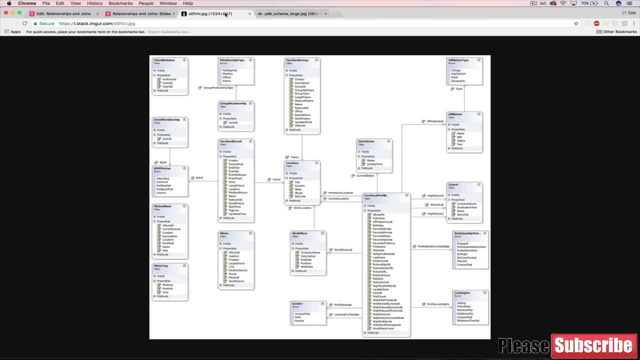 how messy data can be. so here's- I think I showed this early on in the course. this is just a potential schema for Facebook and it's definitely incomplete. it's maybe a tenth of the number of tables that Facebook has, but you can see, just to store basic things. 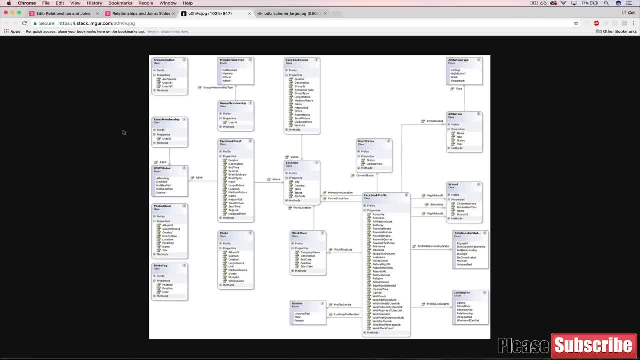 like events and users. we have event Facebook event, we have event membership, which is related to RSVP states, which is also related to venues, which is also related to groups and to workplaces and to Facebook profiles, and it just goes on and on and on. so what I'm trying to show you is that 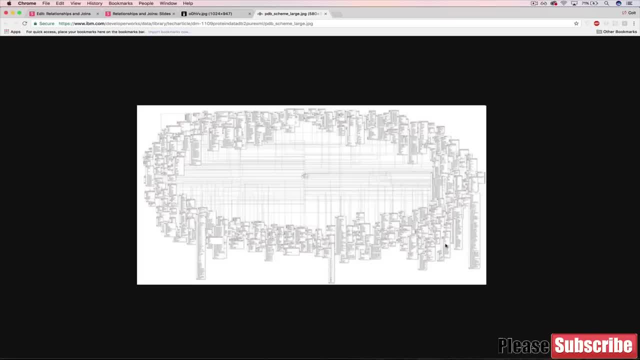 data can get messy and in fact, here's another super intimidating schema. this one is a little bit crazy because it has to do with storing protein database. I think it was. I saw some article on IBM and, I believe, MIT. unfortunately, it's a very 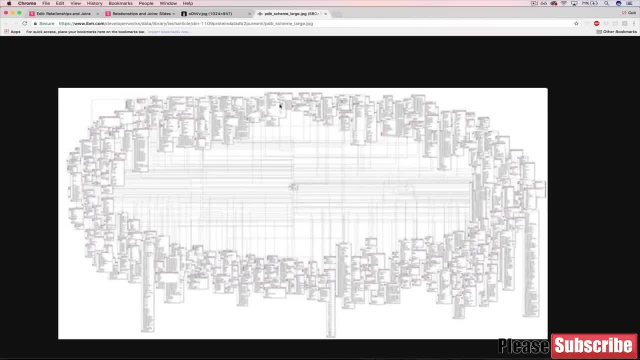 low quality image so you can't actually see the tables, but each one of these little rectangles is a separate table and every line is a connection between the tables. now, this is the worst I've ever seen, the craziest, and I think that was the point. 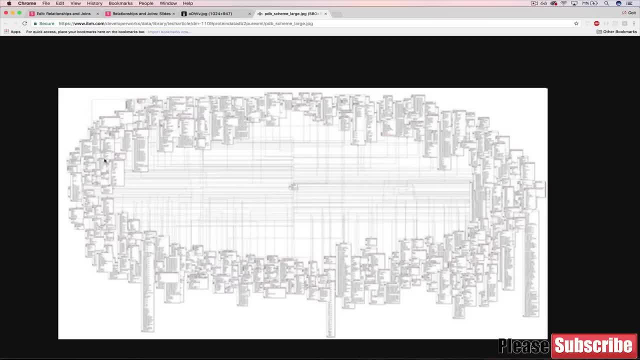 they're trying to just show you. they're never going to actually look at this to try and understand anything, but they're trying to show you how complex protein information is when you have all these different combinations and permutations for a given protein, without going into too much detail here. 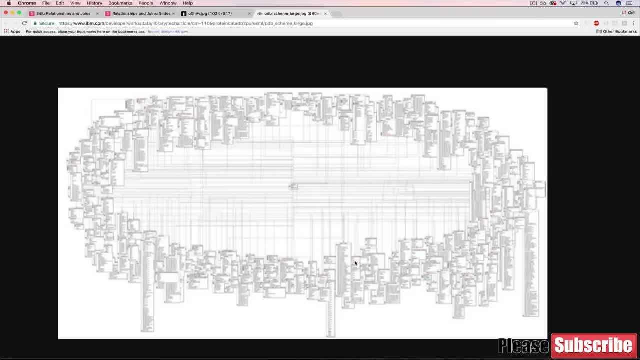 this isn't a bio course, but the way that a protein is folded, the same structure, basically the same amino acids- depending on how it's folded, can drastically change the features, if you will, basically what the protein does, how it behaves, and so this is a way of 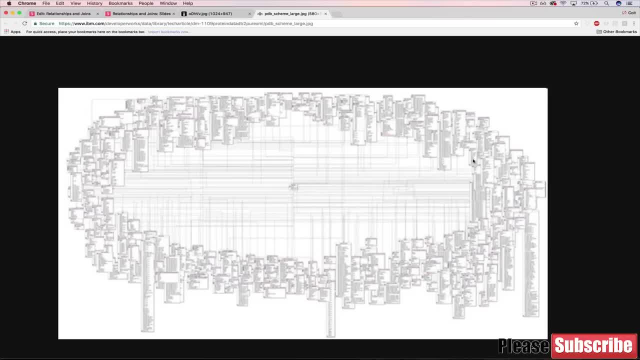 documenting, using SQL in some way, the structure of a protein using a database. okay, so not to scare you there, I just think it's kind of a powerful image, although grainy. it is powerful to see basically some really messy ugly gross data that can be supported. 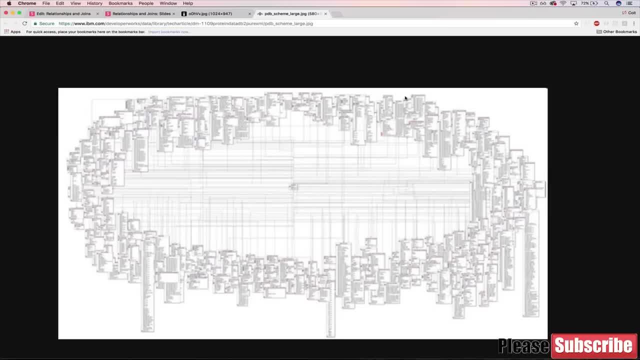 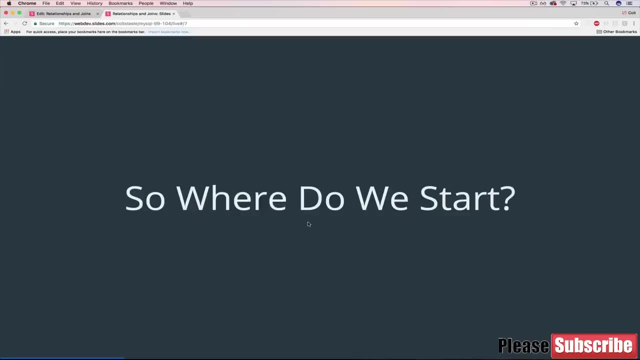 using tables. it just doesn't look pretty. but that's the important part and kind of the point of this video is: I wanted to get you prepared mentally for working with some more complex data, although nothing that looks like this. Okay, so we've established. 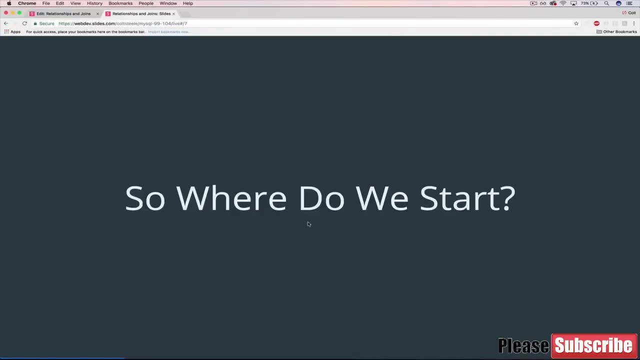 that in real life, data can be crazy complex. outside of the classroom, things aren't as nice as we'd like them to be. so we've established that fact. but now where do we start to kind of wrap our heads around how we represent complex data? 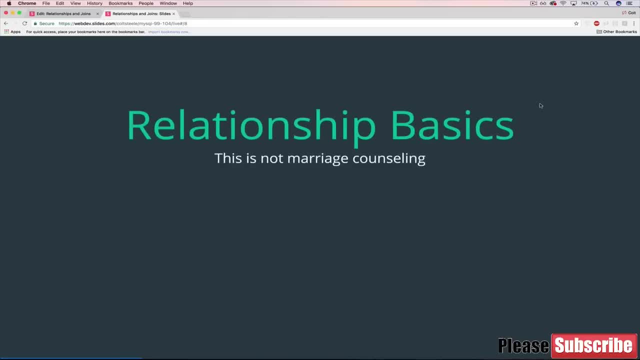 using MySQL and the answer is we're going to start by talking about the relationship basics. so I know it sounds like you know marriage counseling 101 or something, but this is not that. this is about the different ways that data can be related. so if we have two tables, 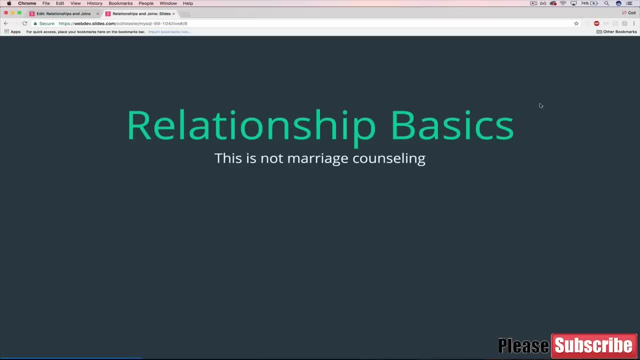 or two entities, things like orders and customers, students and teachers, movies and reviews and users. how are they related? And there's a couple different ways. there's kind of these big, broad categories we can break relationships down into and the terms that I'm 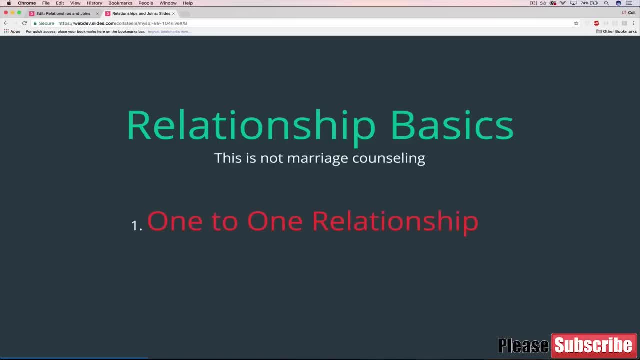 going to use that you'll occasionally come across are three. there's the first one, which is a one-to-one relationship. I'm just going to go through all of them first before we talk about what they mean and talk about examples. so a one-to-one. 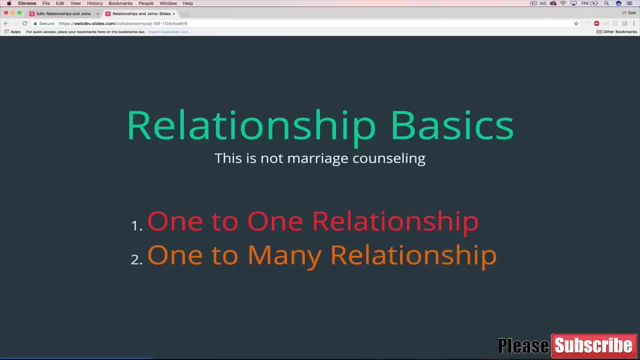 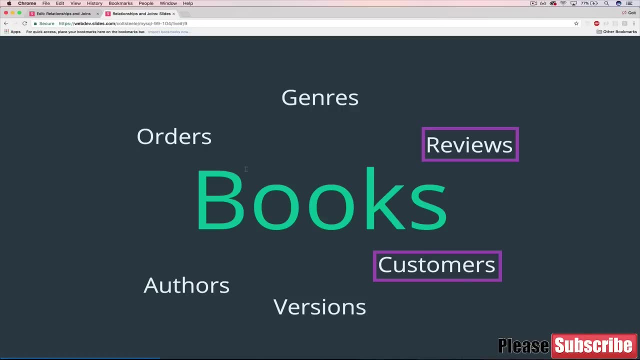 relationship, a one-to-many relationship and then a many-to-many relationship. so the reality is that one-to-one relationships aren't actually that common, but perhaps another example, or one that I've recently used, is I had a customer's table that had the basic information. 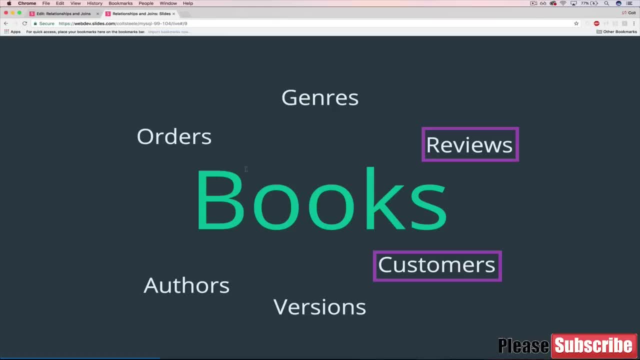 for a customer, so things like their username and their password- although again, you don't actually store the password directly- but username and password and email and registration date. and then there was a separate table where we stored all these details about a customer. so rather, 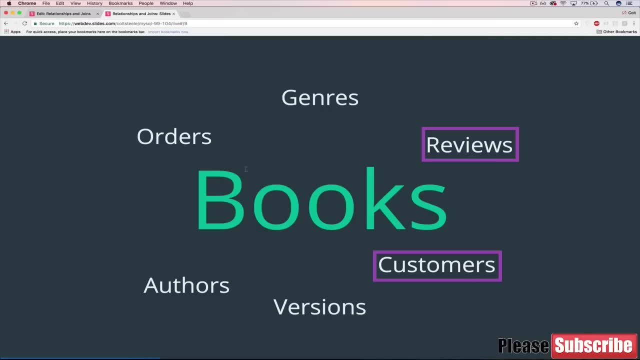 than storing 10 or 20 extra columns on the basic customer table, we decided to split it up based off of what was most commonly needed in the app we were building, and most commonly all we needed was the username and the password and the email, but there was a whole bunch of other information. 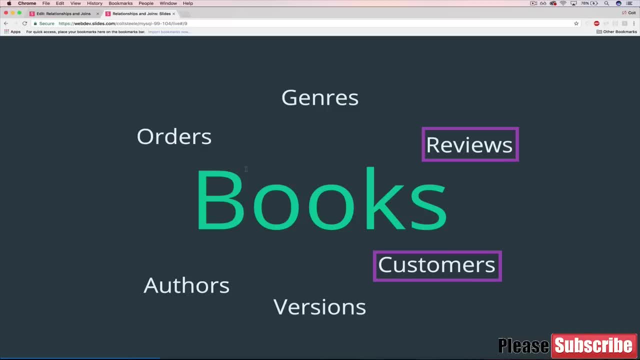 that we were storing. so we created a customer details table and that's a one-to-one relationship. one customer has their own row, one row in the customer details table and one customer details row is associated with one customer. so Colt Steel has a Colt Steel customer details. 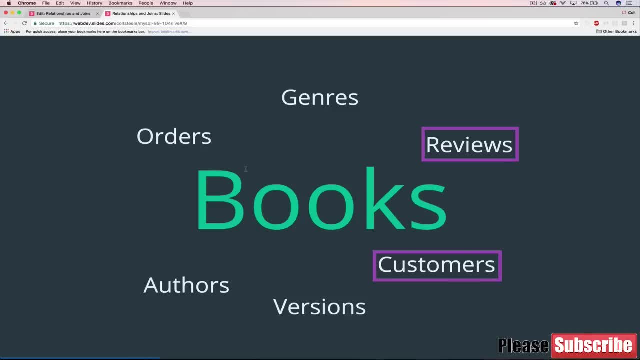 but there's no other user or customer that could be associated with it, because it's a one-to-one relationship anyways. like I said, it's not the most common. what is the most common is actually a one-to-many relationship, and that's what we'll spend the most time on in this. 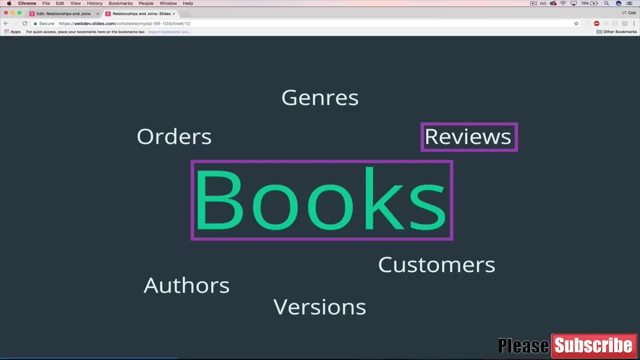 course, because, like I said, it's really common. so here's an example: the relationship between books and reviews. one book can have thousands of reviews. let's say, Into Thin Air by John Krakauer could have probably tens of thousands of reviews by this point. it's been out for a while. 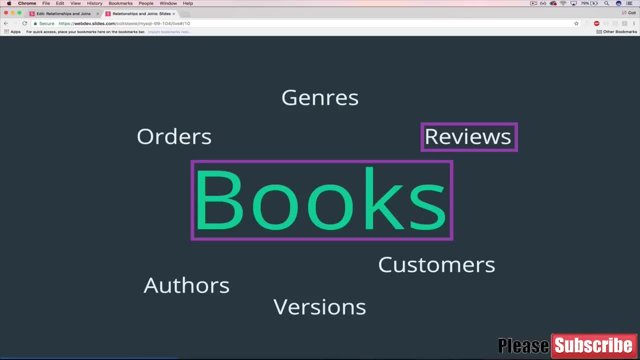 it's pretty popular, but those reviews belong to that book, exclusively to one book. so the relationship is: books have many reviews, but reviews belong to one book, so it's a one-to-many. that's a really common classic example. reviews are ratings and books are some entity. 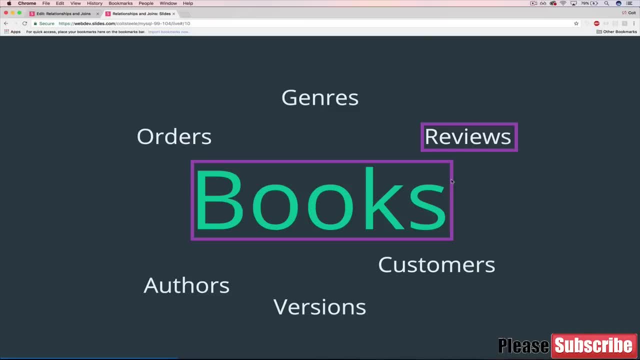 okay, so then the next thing that we'll discuss here is a many-to-many relationship, and many-to-many is still relatively common, and the way that it works is what it sounds like. we have two entities, in this case, books and authors, and 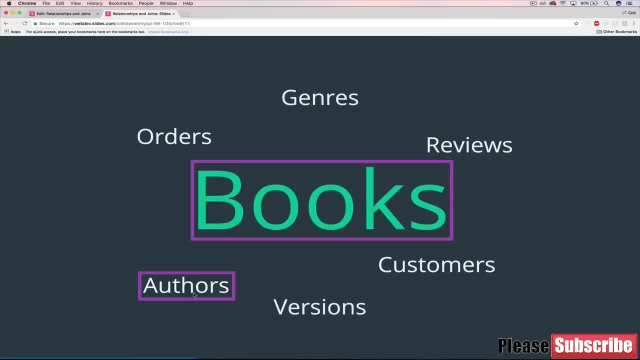 you can kind of speak through it. you can say: okay, books can have many authors, that's true. we could have two authors writing a book together and those authors can have many books. there's no rule that says authors can only write one book. you know JK Rowling. 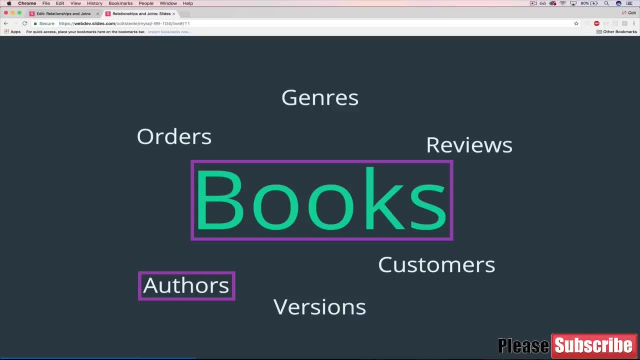 Rowling. however, you say it has ten plus books, so it's a two-way, a many-to-many relationship. so hopefully you can see the difference there. reviews and books- reviews belong to one book. they're associated only with one book, whatever the book title is for that review. 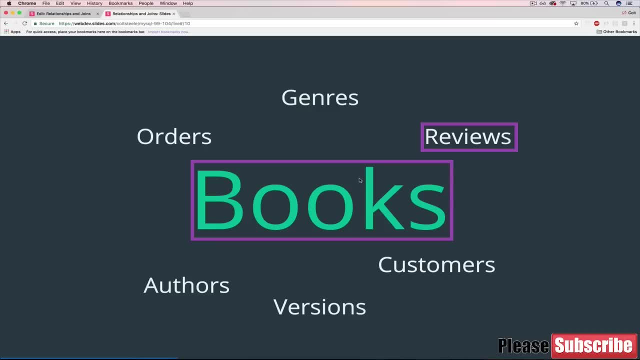 it can't also be the same review associated with another book, so that part of the relationship is one. and then we have the books-to-reviews, which is a many relationship. books have many reviews. this is different because books can have multiple authors and authors can belong to multiple books. 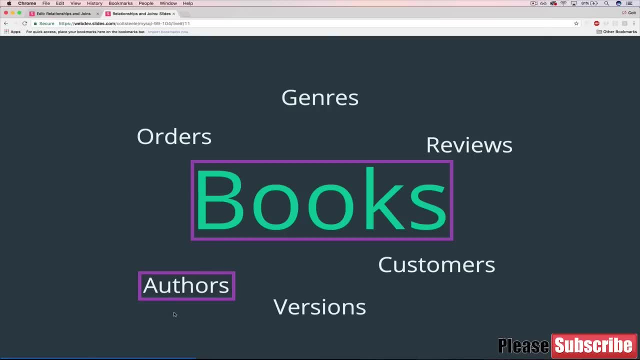 or authors can have multiple books, and the way that we represent this is actually a little more complex. so we're going to come back to it and we're going to start off in this section by talking about the most common relationship and how we represent that which is the one-to-many relationship. 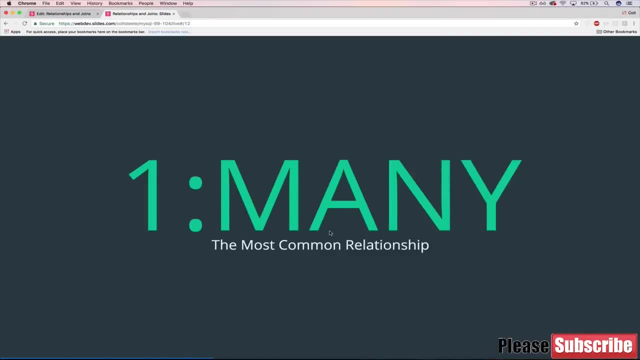 so that's coming up next. okay, so we talked about the three kind of common relationship classifications and, as I mentioned, we're focusing on one-to-many first, and we're doing that for a couple of reasons. one is that, compared to many-to-many, it's a little bit easier to get through. 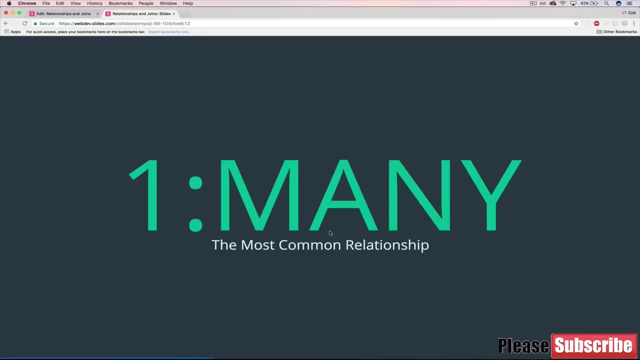 shorter but also it's more common and it's more central, in my opinion, to most of the development that I've done and that I see other people doing. not to discount many-to-many, but we're going to get there. we're starting with one-to-many. 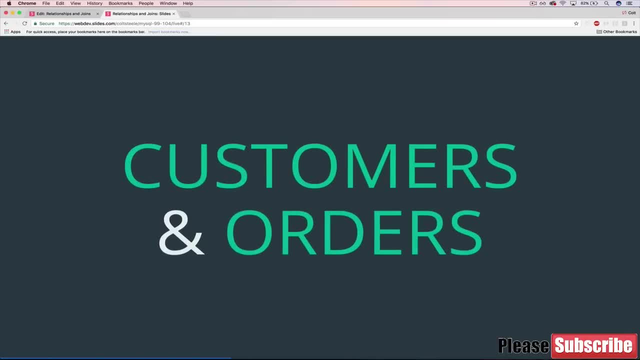 so we're going to start with a classic example: customers and orders, or this could be users and orders, or users and carts, whatever the transaction is, but we're going to call it customers and orders, so two tables and this is a one-to-many relationship. 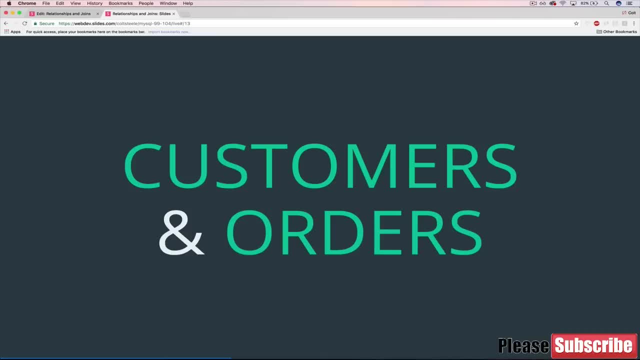 as we talked about earlier. so let's say we have a customer, President Bill Clinton. that's our customer and he can place as many orders as he'd like. he can have many orders, but each of those orders is associated with exactly one user: Bill Clinton. President Bill Clinton, excuse me, 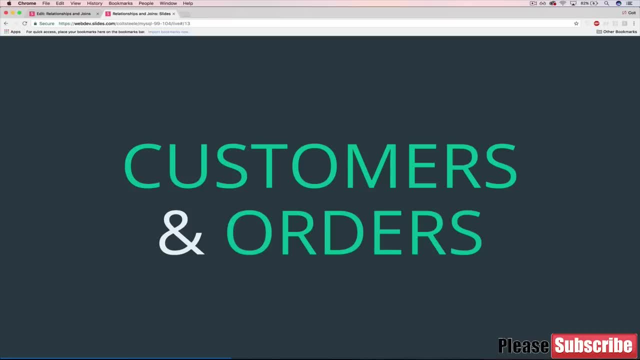 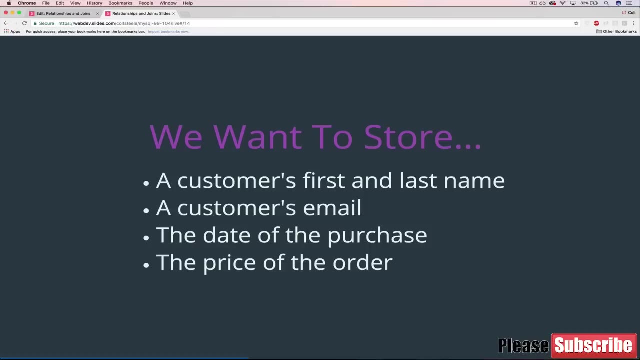 there is no way to have two people associated with one order, so it's a one-to-many. customers have many orders, orders have one customer associated with them, so let's talk about, for our case, what data we want to store, and it's going to be very simple. 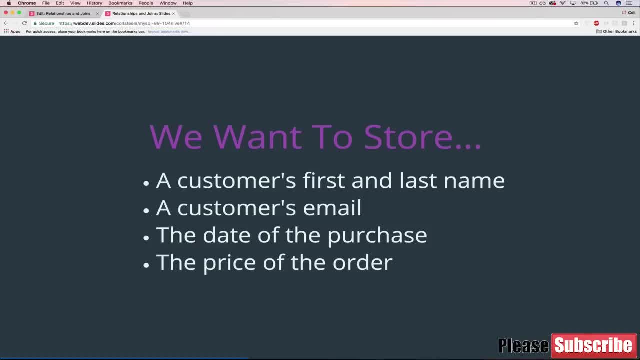 I don't want to clutter it with a whole bunch of other pieces of information. we're just going to focus on the basics. so a first and last name for customers and an email. now, in a real web app, we'd want a lot more information. probably we want to create a registration date. 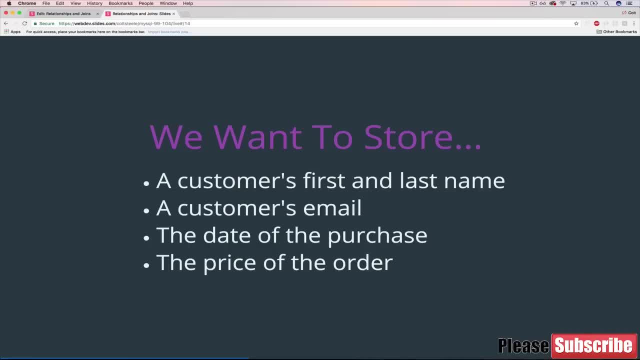 when a customer signs up, maybe a last active date that we're storing, or date time password. somehow we need to store that. there's- I don't know, there's so many other things- phone number if we're trying to do two-factor authentication. 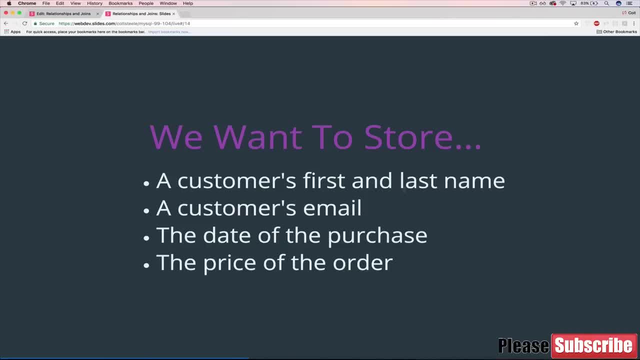 lots of things. so first and last, name and email, so three things per customer. but then we also for orders. we need to store the date that an order was made. so it doesn't matter for our example, if it's date or date time, but we'll keep it simple with date. 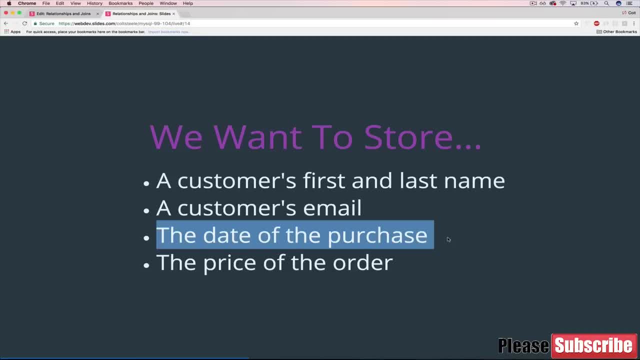 so 2017 slash 11, slash 12 or something, and then the price of the order, the total amount, let's say 99.99 or 20.50. so that's going to be a decimal. so we're going to have first and last name. 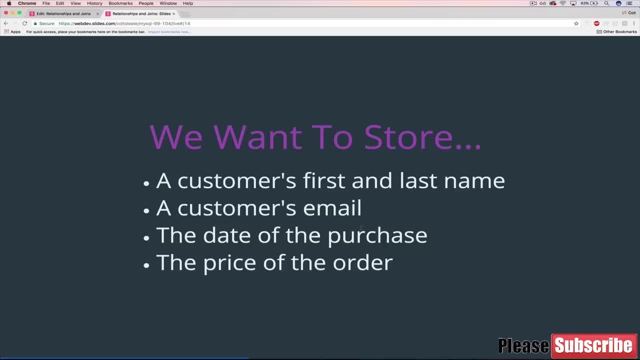 and email, which should probably be varchars, the date of the purchase, which will be a date time, and the price of the order, which will be a decimal. that's the easy part. the next question is: how do we store that? how do we represent it? 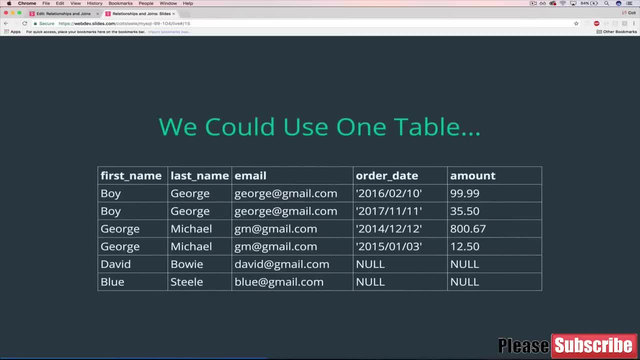 and we could do it this way, which I want to make clear. I'm not saying this is a good way of doing it, but you could technically get away with doing it in one giant table. but there's problems. but let's first just walk through how it works. so we have first name. 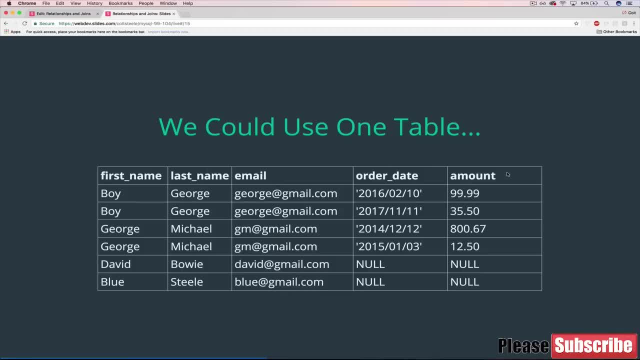 and last name and email for customers, and then order date and amount. so we have, you know, Boy George, who's email is george at gmail dot com. he was a very early user of gmail. and then we have the order date: 2016 to 10. 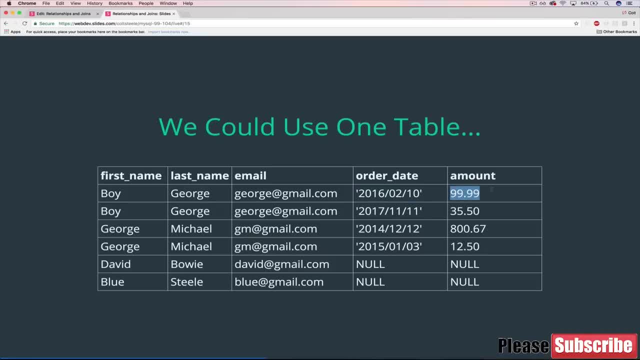 and that order was $99.99. so this is capturing information for one order, but then George, or Boy George, placed another order and we have duplicated information because we're storing. okay, it's Boy George, which I know- Boy is not his first name, but just. 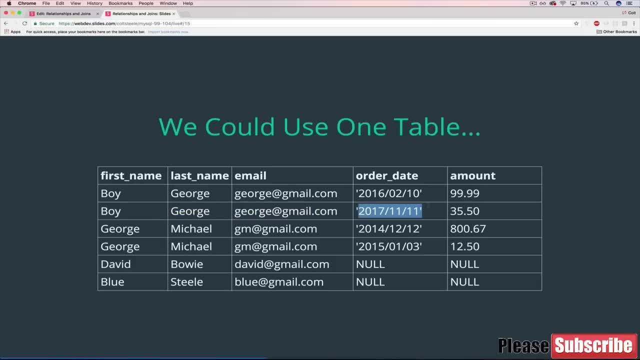 let's go with it. and then George at gmail again, and then a different date- this one was later in 2017, and then a different price or a different amount. so this stores the information that we talked about we needed first last email. 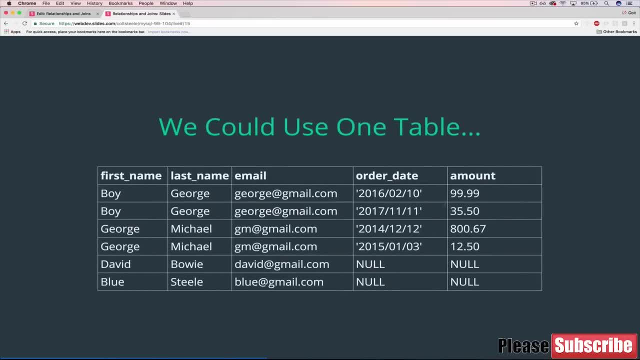 and then date of the purchase and price of the order, and so that's working. same thing with George Michael, who has gm at gmail dot com, bought something in 2014, that was $800.67. and then George Michael, same email, bought something in 2015, that was. 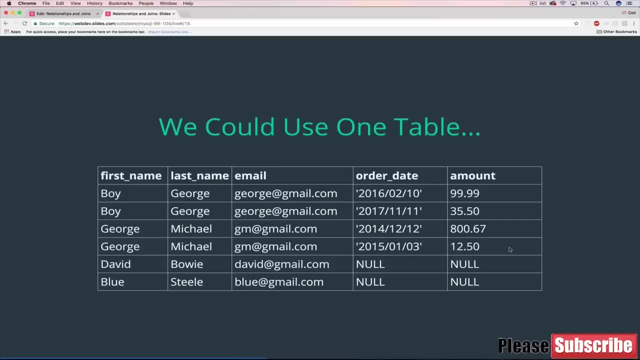 $12.50. okay, so already you should be noticing we have a lot of duplication, right, even though we are storing the information that we're supposed to store, there's a lot of duplicated data. and then we run into these two, David Bowie and Blue Steel- my cat. 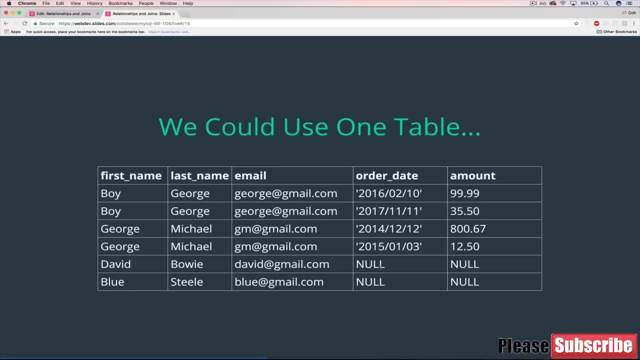 there's problems because they haven't placed orders yet, so we have their customer information. we have David Bowie- David at gmail dot com, also early adopter of gmail, and we have Blue Steel- Blue- at gmail dot com, and they haven't placed orders, but they still have order date and amount. 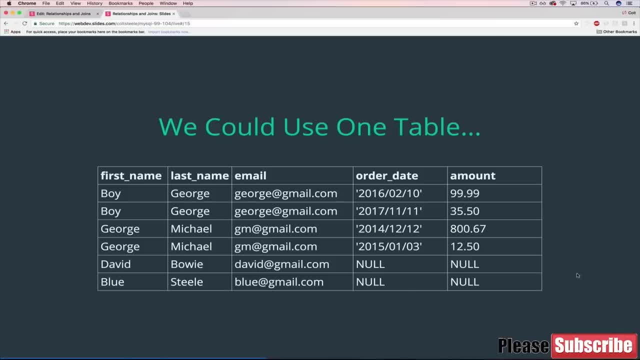 as columns and they just have no value. it's null. so this technically represents that fact that Boy George and George Michael have two orders each and David Bowie and Blue Steel have no orders. so that's really not a great way of doing it. yes, it works, but we're 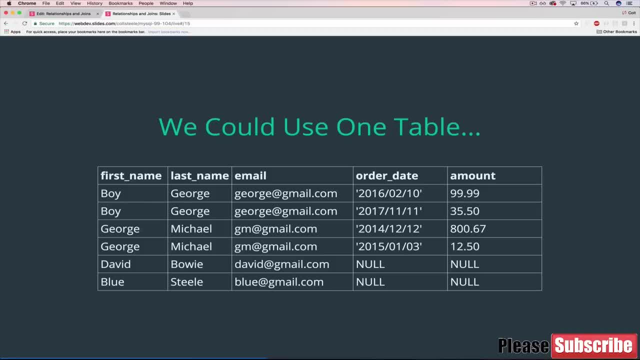 not only duplicating a lot of things- right, Boy George, George Michael, and if somebody shopped a lot, we would have tons of duplicated information, which is just a waste- but then also we run into problems where we have users who maybe haven't ordered anything yet. 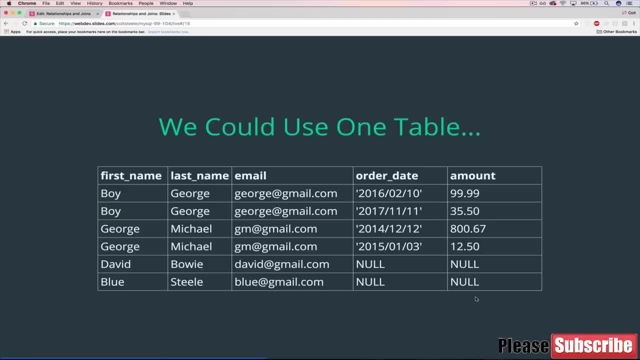 and they just signed up for the site. there's no reason to have anything to do with orders until they actually place an order. so it's much better to keep our data separated, because if we ever need to work with just customers on their own, which is 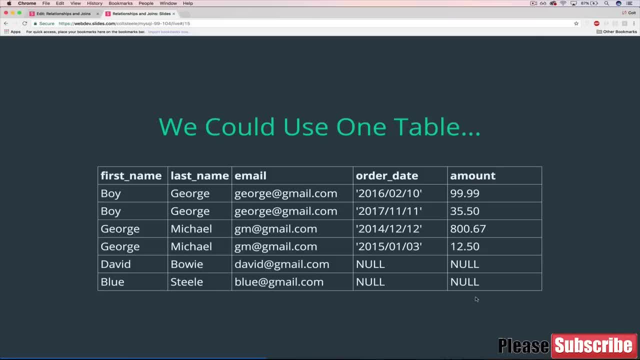 happens. there are times on a site where you don't care about orders, you just care about customers. let's say, when a customer is signing in, all that you need is to take their email and check it, and take a password and check it against. 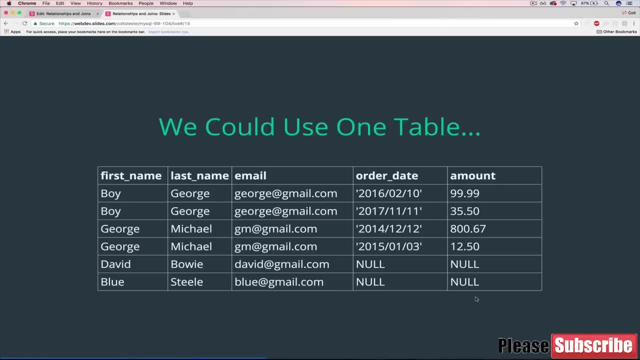 the password field. that has nothing to do with orders, so why would we need to go through a giant customer orders table? and that's just a really silly example. but what I'm trying to show is that it's not just about the duplication. 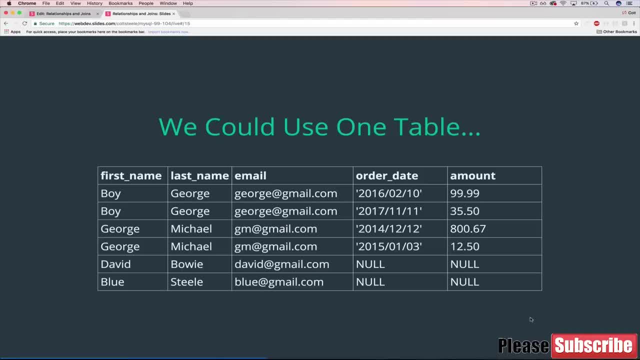 it's also that sometimes it's better to keep your data separate almost every time, unless you're always accessing your data together, like if the only time we're ever talking about customers is when we're talking about orders, then okay, maybe you could put them together, but then we still have. 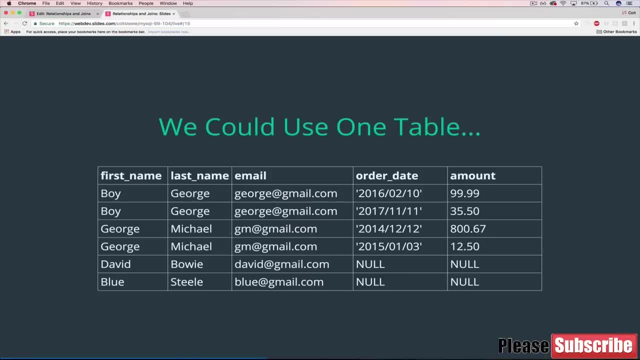 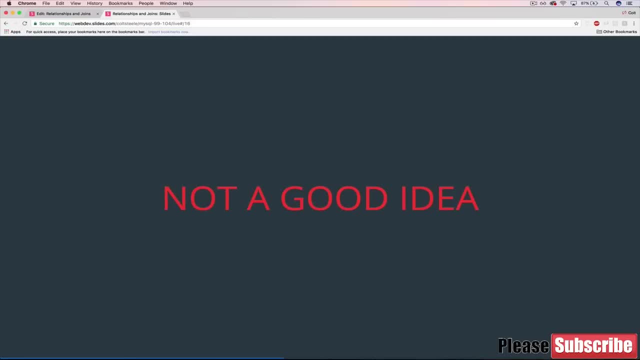 this problem where we have people who haven't placed orders or we have duplicated data. so this is a bad idea, not a good idea, aka bad idea. so what do we do? well, here is the simplest approach. this is how we express. 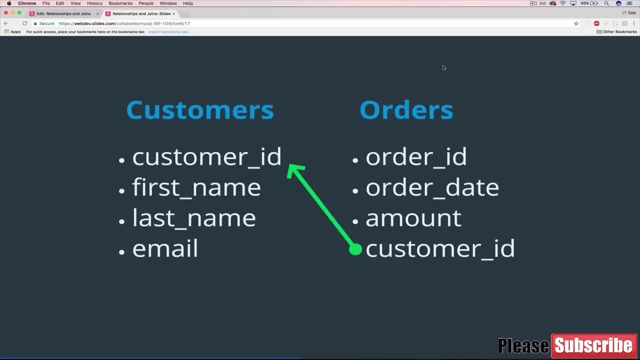 a one to many relationship and it looks like this: so we have two tables: customers and orders. customers have an ID field and then a first name, last name and email, and then orders have an ID field and then the date, the amount and then 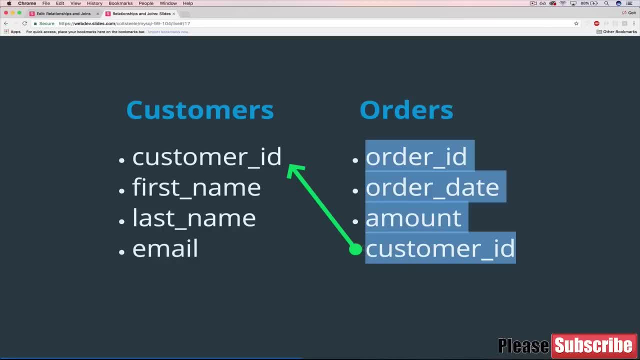 this is the important, this is the crux of everything. they have a field called it. doesn't matter necessarily what it's called, but ours is called customer ID and it's a reference to the customer's table. so whatever customer ID is, 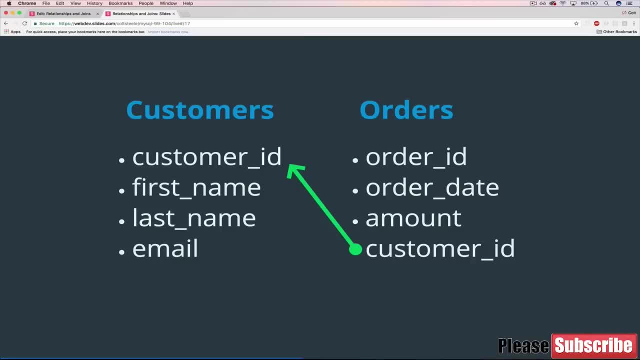 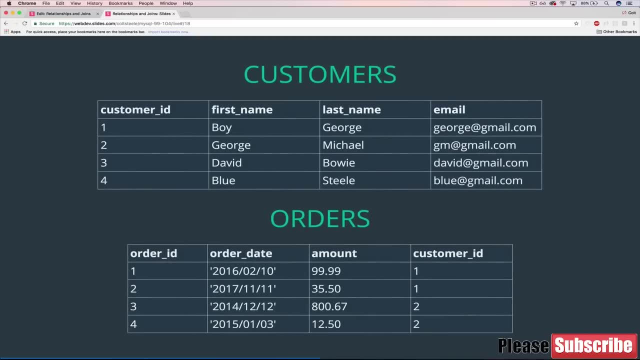 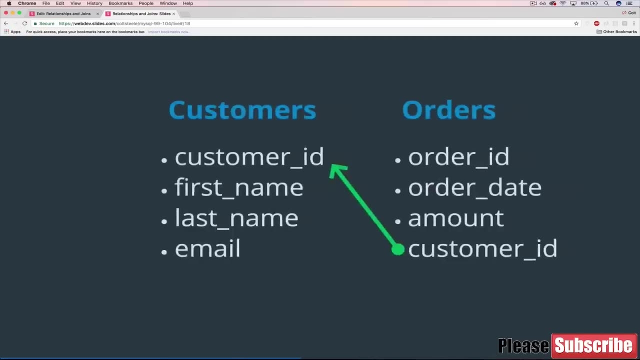 in a given order is going to correspond to an actual customer who placed it. so let's dive into it a bit more. here's an example. so I took the exact same data- we had four orders and four customers from back here and I split it up into separate tables. 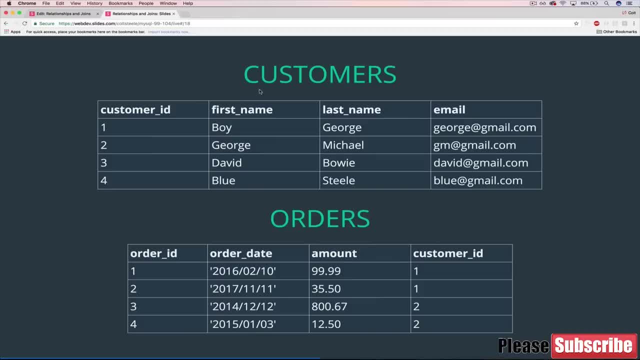 and you can see. let's just talk about customers first. we have a customer's table with an ID, a first name, last name and an email. so we have boy George George at gmail ID 1. George Michael GM at gmail ID 2, David Bowie. 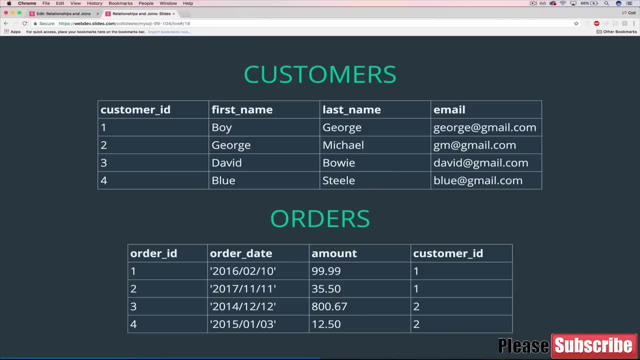 David at gmailcom ID 3, and then blue steel blue at gmailcom ID of 4. these are all unique, corresponding to exactly one user or one customer, and then we have our orders table. so there's an ID there. order ID. 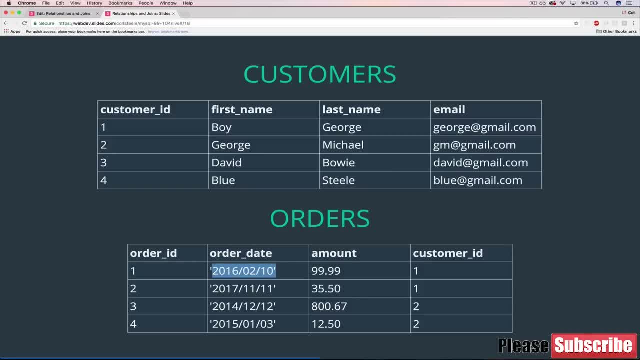 and then the date that an order was placed, and then the amount, and then the most important part- arguably the most important part, definitely the crux of the relationship- is customer ID. so in this case, it's 1 which is pointing to this customer with ID of 1. 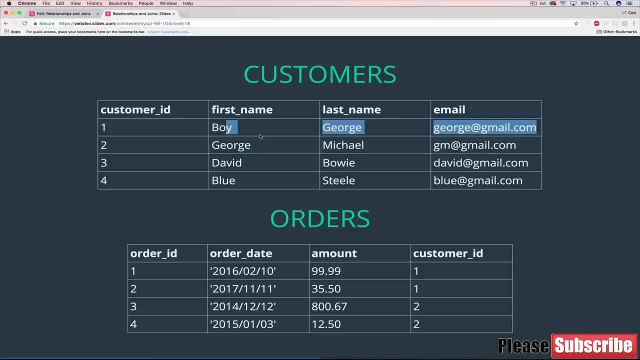 meaning boy George. so boy George placed an order in 2016 for $99.99. here's another customer ID 1 telling us that this entire row here, this order, is related to boy George again. so he placed an order for $35.50 on 2017. 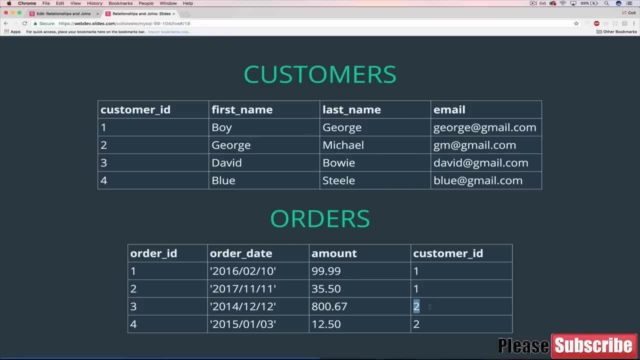 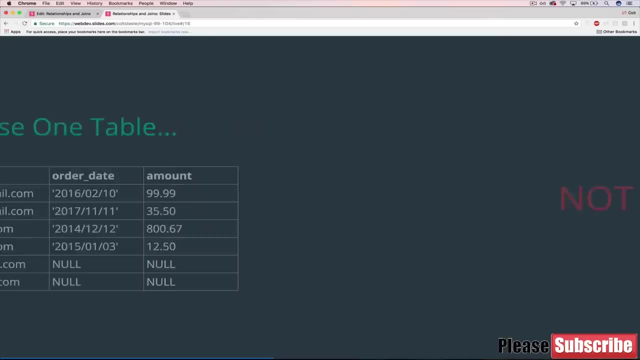 and then we have George Michael, customer ID. 2 matches this ID here and he bought something for $800.67 in 2014 and something in 2015 for $12.50, which is the exact same data we had represented here, and then notice that we have users. 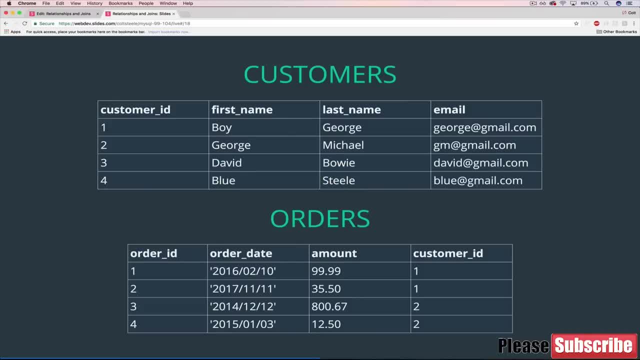 like David Bowie or customers- excuse me, David Bowie and Blue Steel- who haven't bought anything, and there's no extra data, there's no nulls. we have the minimum information that we need. we're not storing anything that we don't need, so we don't have. 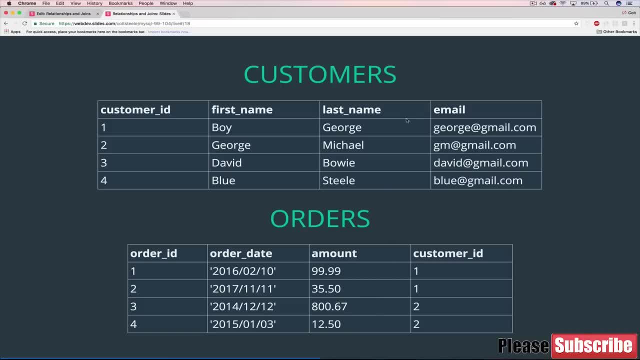 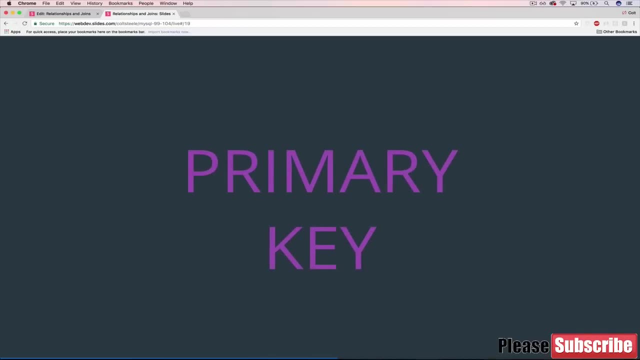 extra orders that are created because they haven't created orders. we have separate tables and we also have other tables that we don't use, like we have in the context of Burn-out Street. this is the classic way of structuring a one-to-many relationship. 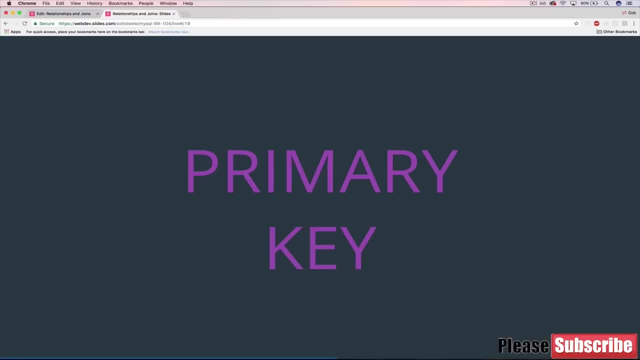 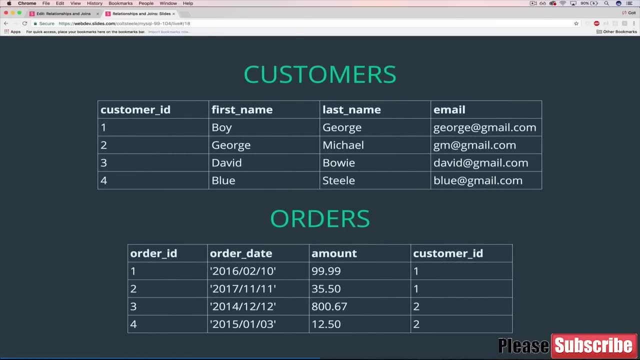 and, along with that, there are 2 terms we need to point out, which we have briefly discussed, and the first one is primary key. so remember this keyword we can type when we're defining a schema. we can say: and what we've been saying, a lot is ID. 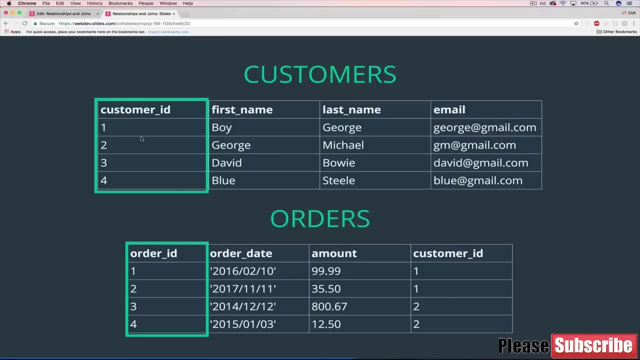 space Int is always unique. So we only have one customer with ID of one and only one customer with ID of two and three and four. And that's really important because if we're referencing it somewhere else, like over here, if there are two different customers that have ID of one. 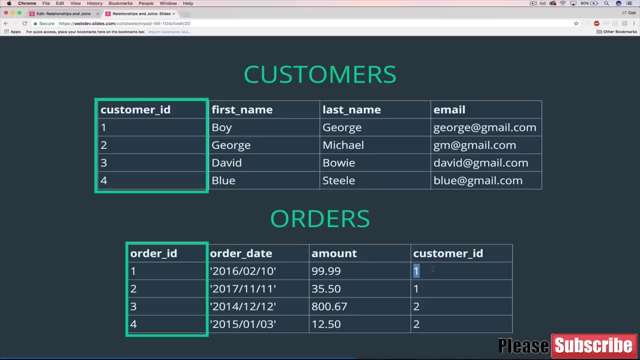 then this is useless, because which one does it refer to? So it has to be unique. And then that's where the auto increment comes in right, Where it will make it unique. every time we insert a new customer, it will automatically increment this to five and to six and to seven. So there is no. 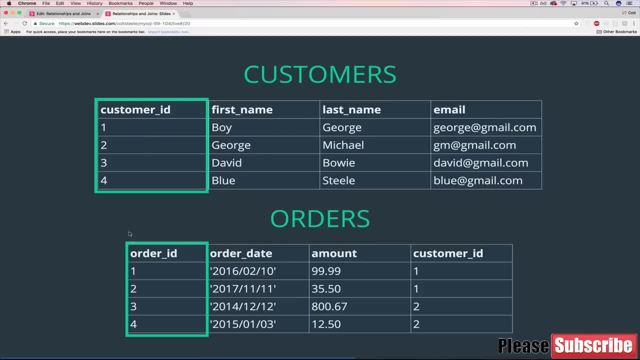 possible way we could have duplicate customer IDs. And then also here is order ID, which is also a primary key. It is the way, the unique way, of referencing an order. Now, this is a bit extreme, but it's possible that we would have two duplicate rows here where basically an order was. 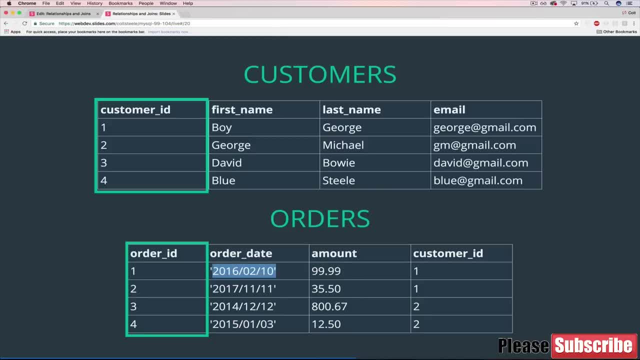 placed for the same amount at the same day by the same person. It's possible And we would need to refer to them separately, though We don't want our database just to combine them. Maybe a user purposefully bought the same thing twice. They bought it once and then. 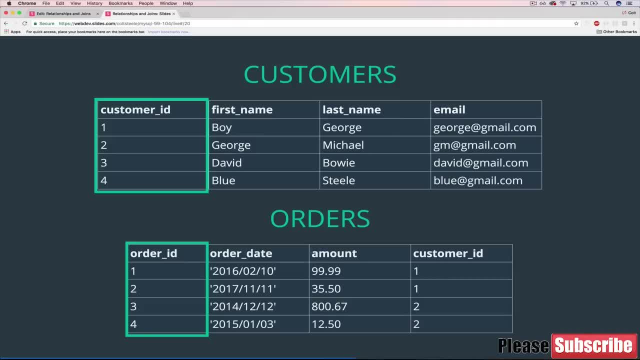 they realized, oh shoot, I really should have bought two. So then they buy it again: same amount, same day, same customer ID. Well, the only thing that keeps those orders unique is our order ID. So again, these two are primary keys. They are the primary way of referring to rows in this table. 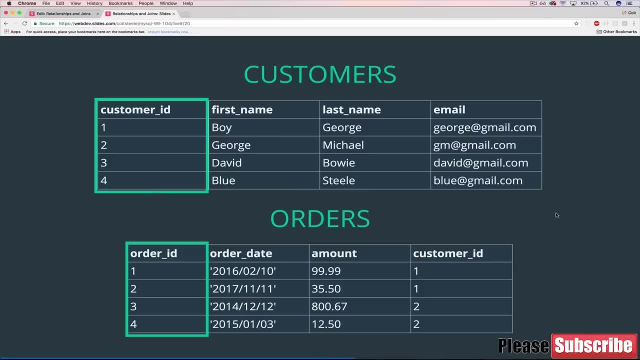 It's what makes them- or it's not the only thing that makes them unique, but it is guaranteed to be unique. And then that brings us to foreign keys, And foreign keys are references to another table within a given table. So in this case, in our orders table customer ID is a foreign key. 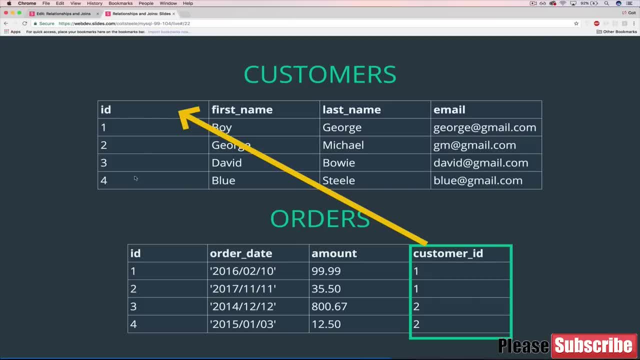 because it's referring to this ID of the customers. So primary key, primary key, foreign key, Customers- does not have a foreign key in it. It's not referring to any external table, but orders has a foreign key And that terminology is important. We'll come back to it a lot. 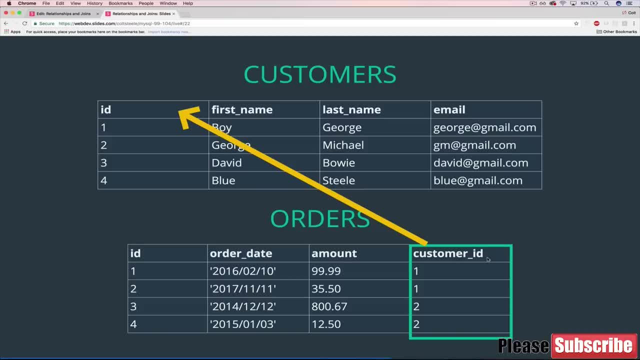 Primary key and foreign key. It'll also show you how you actually say in your schema definition that something is a foreign key And the reason you would do that is to enforce that whatever customer ID is in here is an existing customer ID over here. Because what if we inserted something? 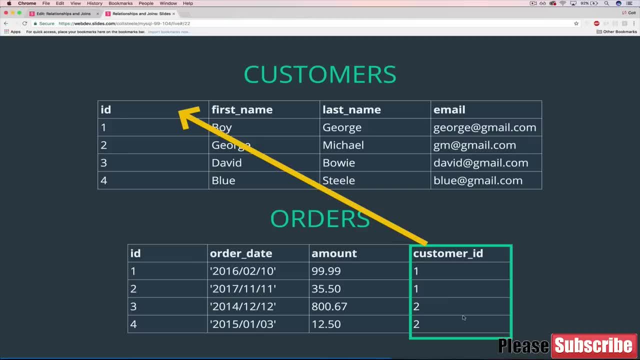 an order amount with customer id of 20 and we don't have a customer with id of 20, we may not- i mean most likely, we don't want that to happen, right? we would want to bounce that back and say, hey, this is a problem, there's not a valid customer with that id and that's what foreign key when we use that. 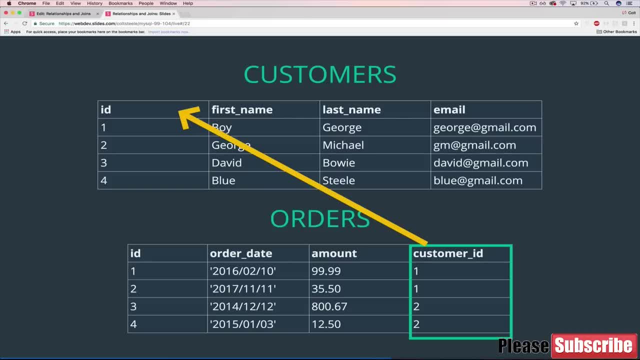 in our schema definition, it will enforce that. otherwise, if we don't say that it's a foreign key explicitly, we could have customer ids, you know, all over the place that don't actually exist. okay, so this is the schema that we've defined. well, this isn't the actual schema, but this is the the. 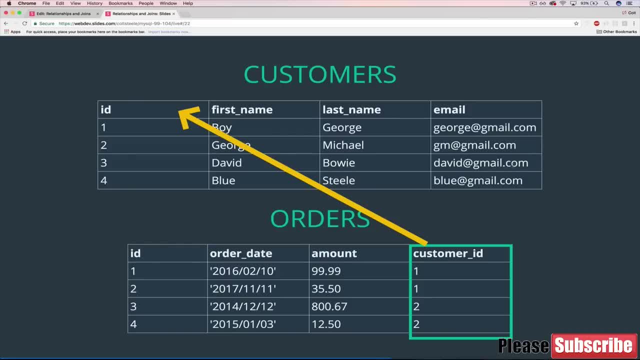 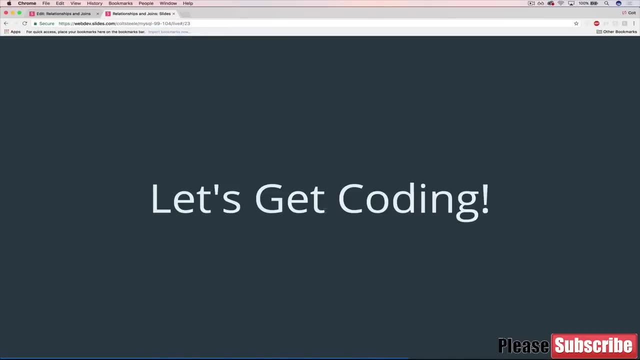 basics of what we want our schema to look like. now we're going to implement it in the next video. all right, so we discussed our game plan for implementing the relationship, the one-to-many association between customers and orders. now let's get to it. so we'll start off with customers. 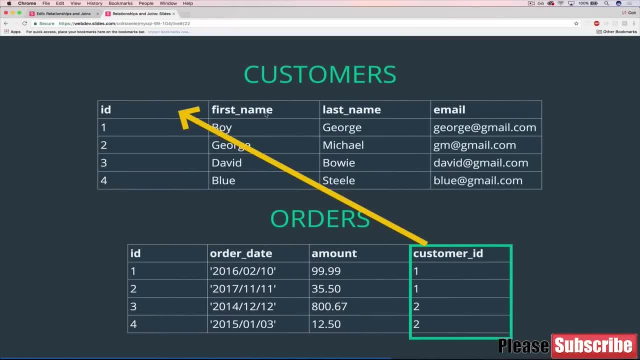 which is a little bit easier. so we're going to have an id, a first name, a last name, an email and these three- the last three- are all var charts. an id is an int, so let's start off with that and i'll let you know. you know, i have basically our 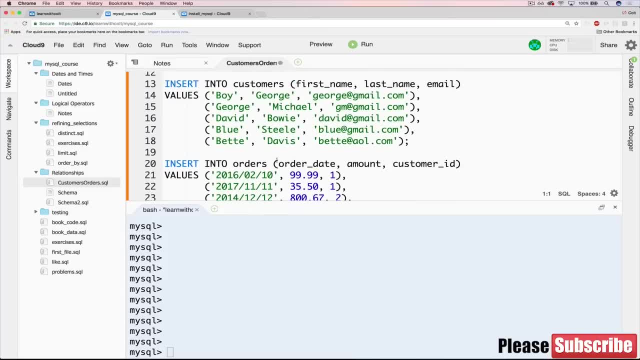 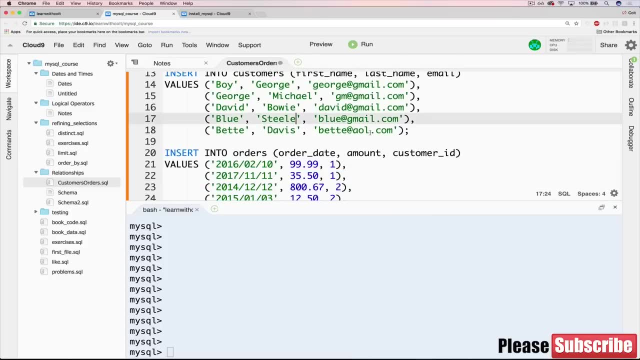 data already written so that we don't have to spend time typing it out. you'll be able to copy and paste it, but i do think it's good if you go through actually typing the schema itself and just copy the copy and paste the data in, because there's no reason you need to spend time. 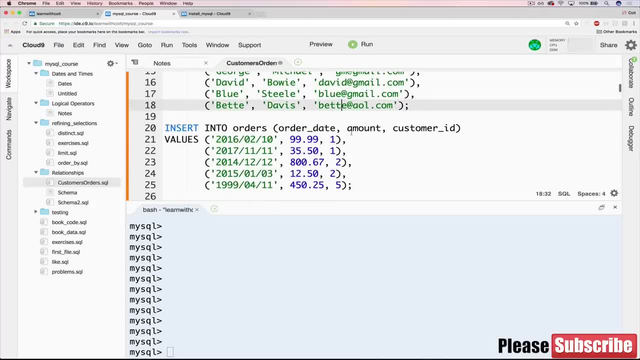 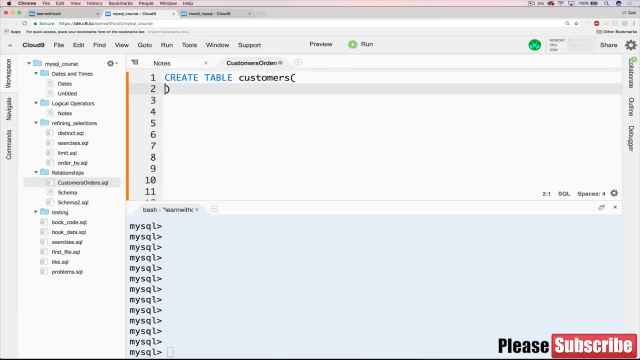 you know typing blue steel and all these email addresses over and over. okay, so create table customers and let's just start by defining what we need. so we have an id, we have first name, we have last name and we have email and, as we said, these are all var chars and we'll just do 100 and i'll copy that. 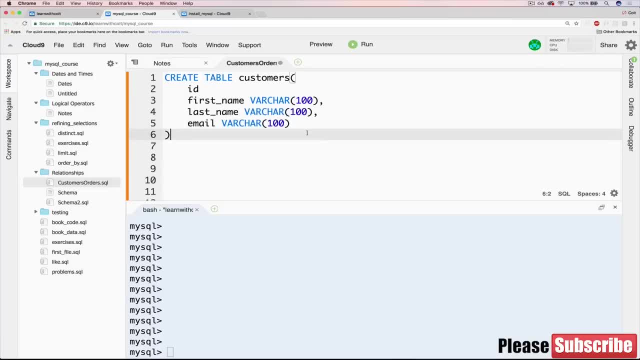 and paste it, add my semicolon, and so we're almost there. we just need to figure out id and this should be review. we have int and we could leave it at that, but it's best to add auto increment and primary key, and that's because, well, a couple things: one: 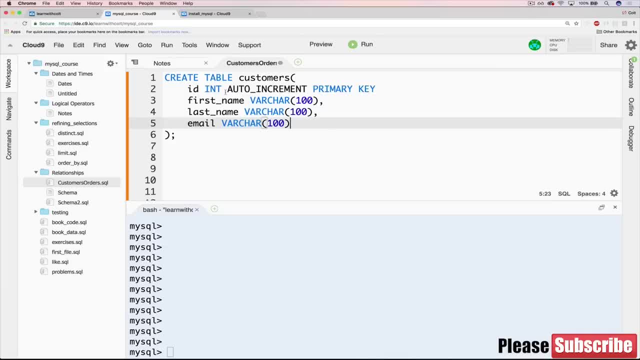 it's a good habit to get into. at the very least it can be useful for sorting things. but, more importantly, we are going to reference this id- customer's id- in another table and so we want to make sure that it's unique, like we discussed. we don't want to have you know customer. 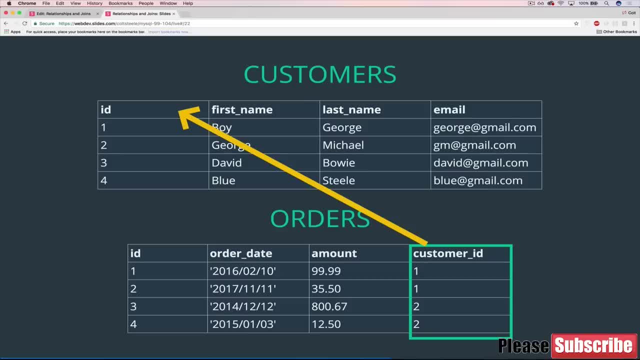 id too. we don't want any ambiguity as to who or which customer that's referring to us so we're referring to. if we had two different customers with the same id, that would be problematic, so we're going to make it unique with auto or with primary key and auto increment. now primary key on. 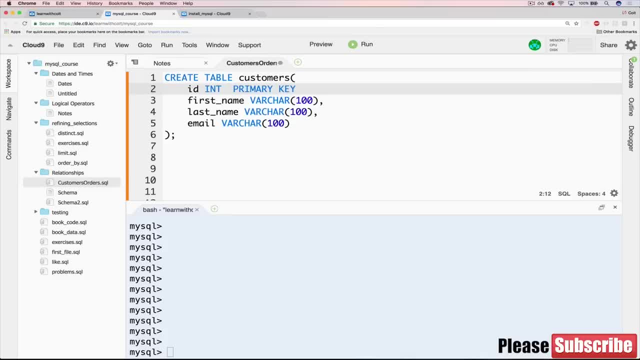 its own enforces the fact that it's unique, but we would have to manually enter it in. it should be review, but i would have to actually say something like insert into customers, and then what would i do here? let's say id and i'll just do first name. 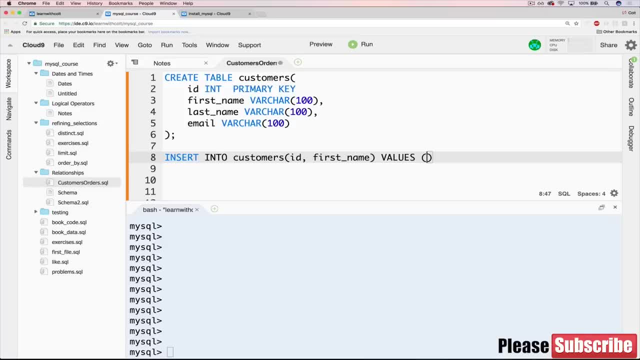 i would have to manually go through and say, okay, this user has id of two and a first name of tom and then the next one. i would have to make sure it was unique and do three, or i could do 20 or 50 as long as it was unique. but i don't have to care about that id if i put auto increment, so we'll do. 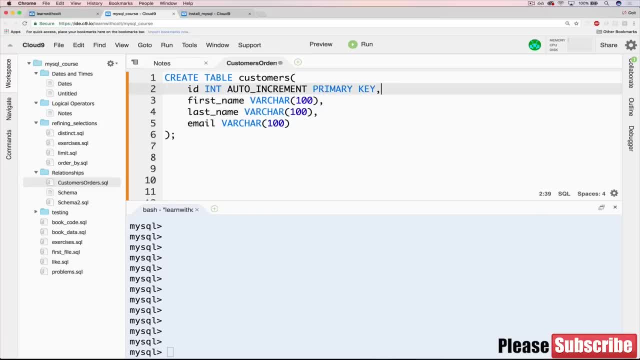 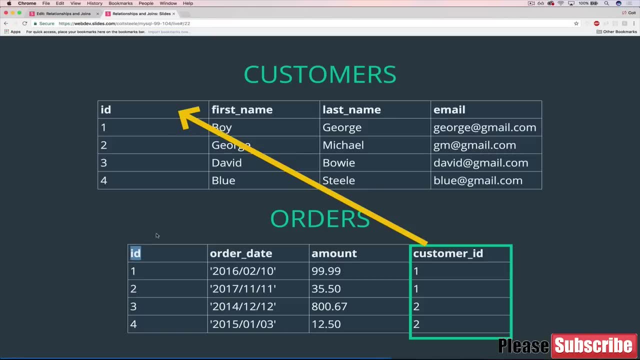 that okay. so that gives us customers. let's make sure we add our comma there, and then next up we have orders, and order has an id as well. so that will also be the first order, and then we have an order key. so that's basically what's going to make this work. 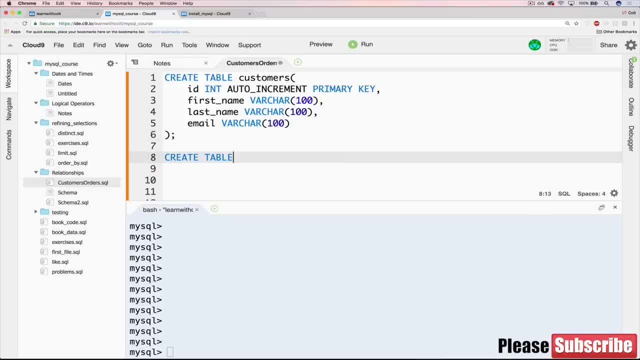 and then we have order, date and amount. so let's start with those three, create table orders and the first thing we have is id. and then we had order date and you might be inclined just to call it date, but that can be problematic because that is an actual data type. it would be like naming a 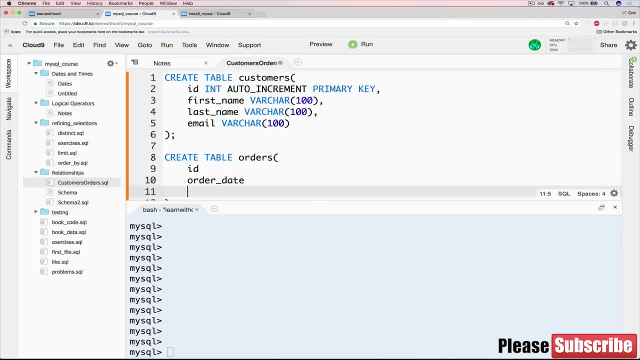 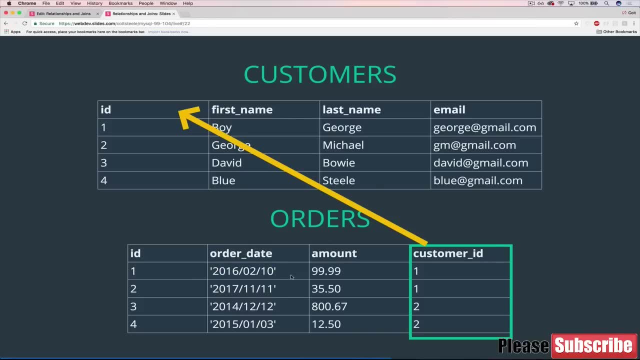 column int or var char. so we don't want to do that, so we'll call it. then we have amount. Okay, so order date: it's just going to be a regular date. we won't worry with date time, even though I prefer date time, Just to make it simpler for us. we won't have to. 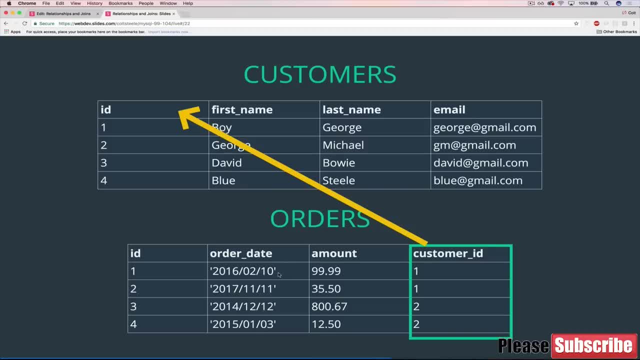 deal with the time component. So that's not what this is this exercise is focused on. So we're just going to eliminate that. So date, and then this will be a decimal, And for our purposes let's say eight comma two. So we're: eight is the total number of digits and two is the number after. 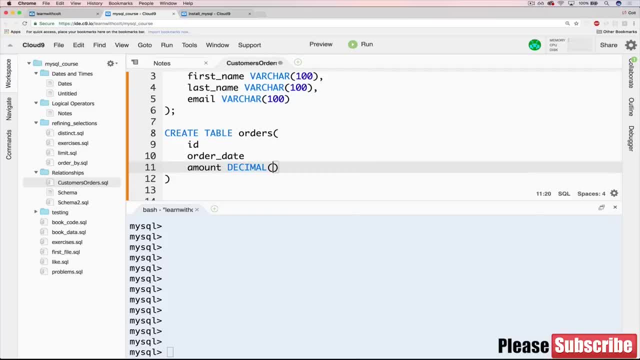 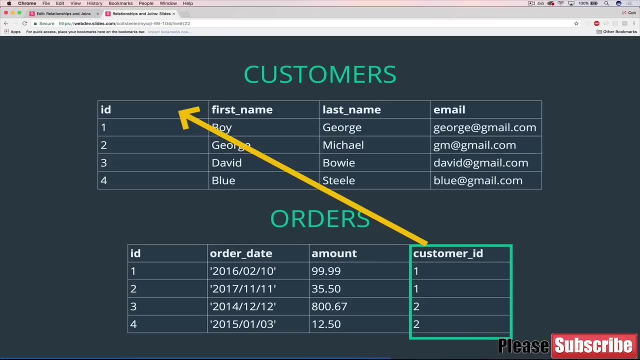 the decimal, So we'll start with that decimal. eight comma two: Order date is just a simple date, And then ID is an int And we'll do the same: auto increment, primary key. But then that brings us to the last thing, which is different. We haven't seen this before And all we're going to do is 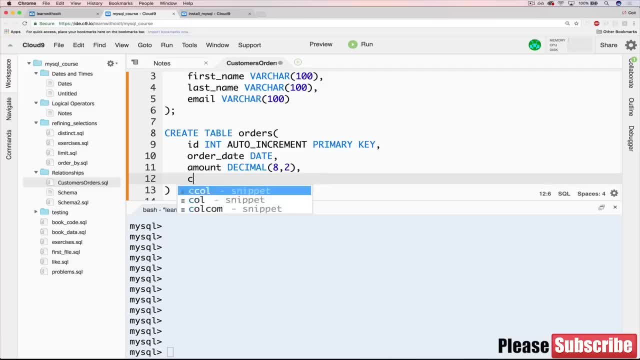 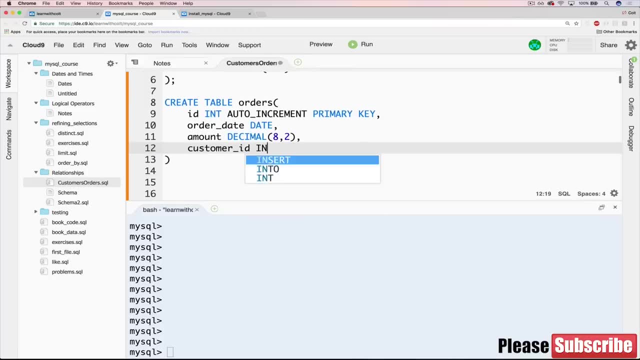 write customer ID. That is the name of the column. What data type is it? Well, it's just going to be a number, it's an integer, So we could just leave it at that if we wanted to, And I'll show you what that looks like to start. So I will go ahead and leave it at. 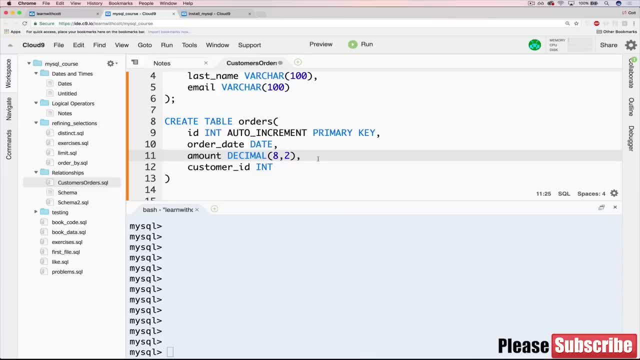 this. I'm not recommending that you actually run this just yet, because we are going to change this, And I'll show you why in just a second. Okay, so let me add my semicolon in here And then let's make sure we don't have any typos. The first thing I'll show you is that I'm in a new database. 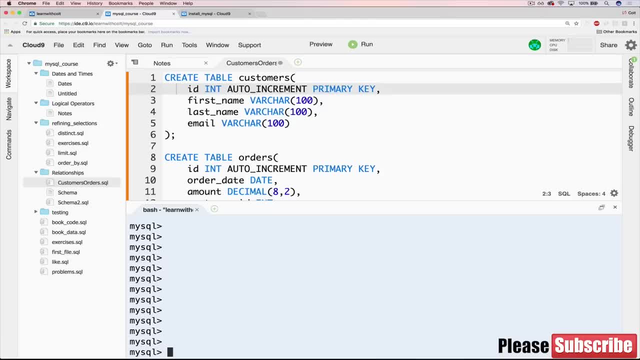 It's been a bit of a review, but it's been a while. How do I check the name of the database that I'm currently in It's select database? So I made a new one. It doesn't matter, You could do it inside. 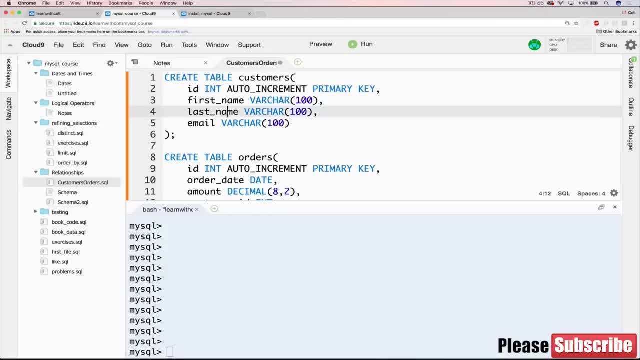 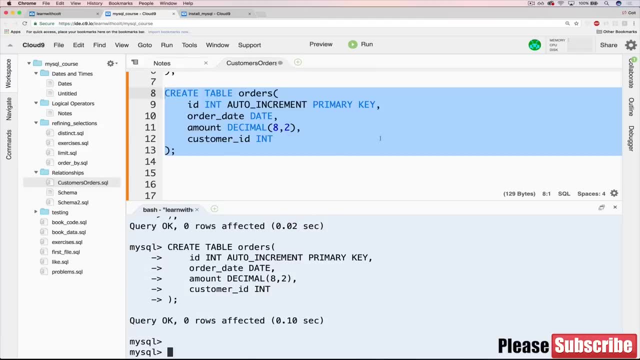 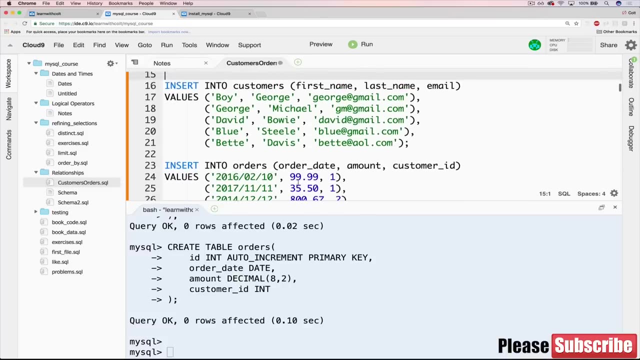 the bookshop. I just wanted to have a clean thing. We have no tables yet, So I'm going to make our customers table and see if it works, And then our orders table. Okay, perfect. So then I have all of this data down here that I'm not going to type by hand, So I'm going to make a new one And then I'm 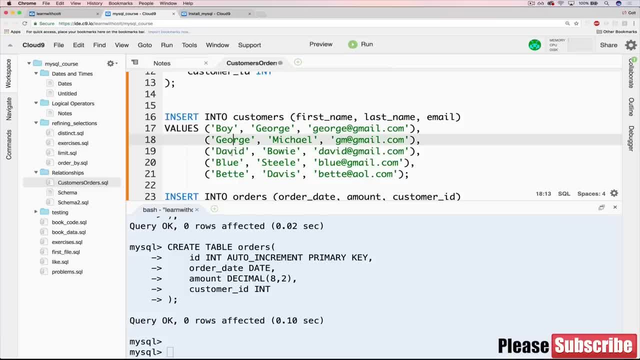 going to make a new one, And then I'm going to make a new one, And then I'm going to make a new one. But if we take a look, it's adding how many users? Five users. I added one who wasn't in our. 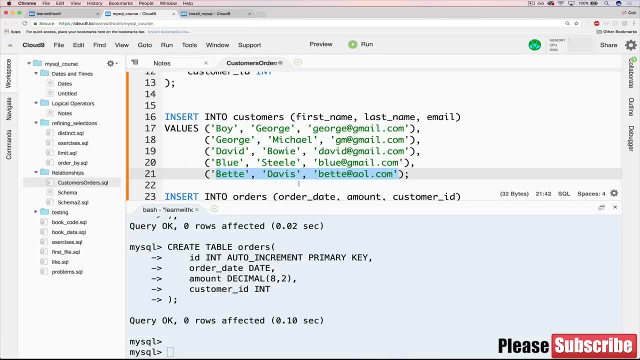 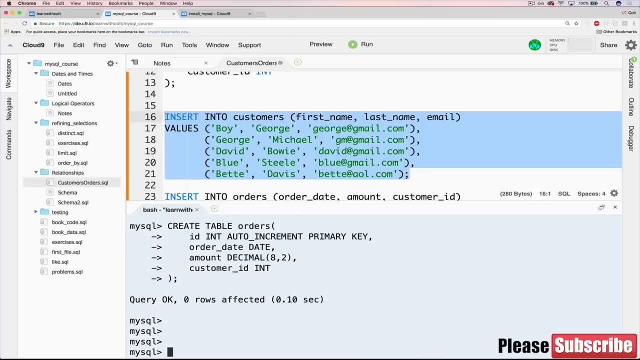 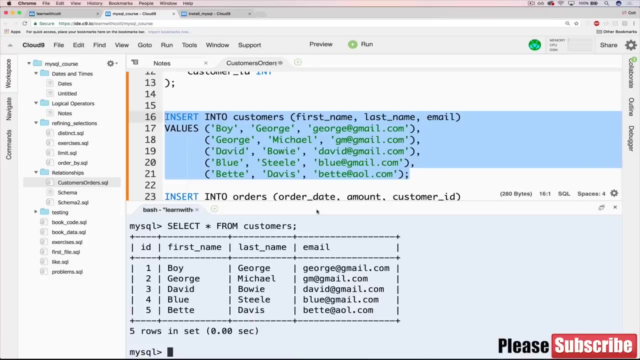 database already, or who wasn't on the table here, which is Betty Davis. So we have Boy George, George Michael, David Bowie, Blue Steel and Betty Davis, So that's just going to insert into customers. Make sure that works. Let's do a select star from customers- Perfect, And then this is a. 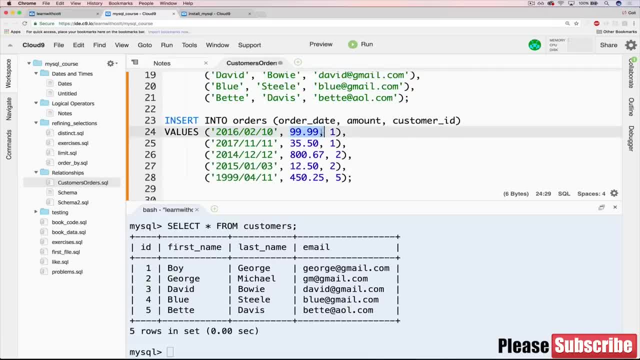 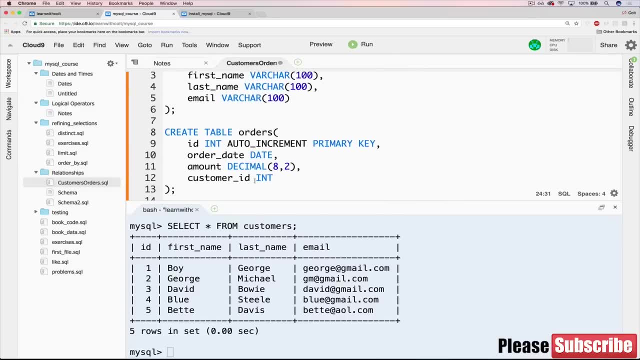 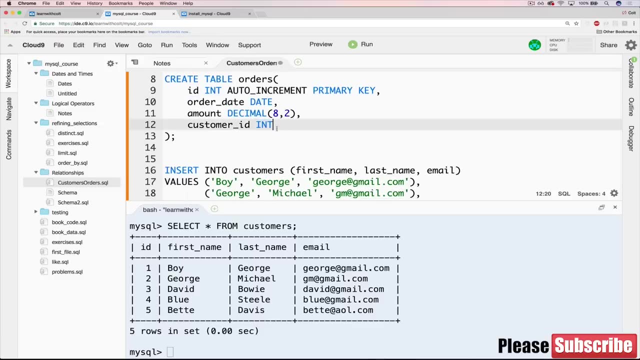 notice. all that I'm doing is the date of the order, the price and then customer ID at the end, And right now there is no explicit association between customer ID here and ID here. All that I've said is: this is a number, So it's up to me to put whatever I want in there. So let me show you. I'm 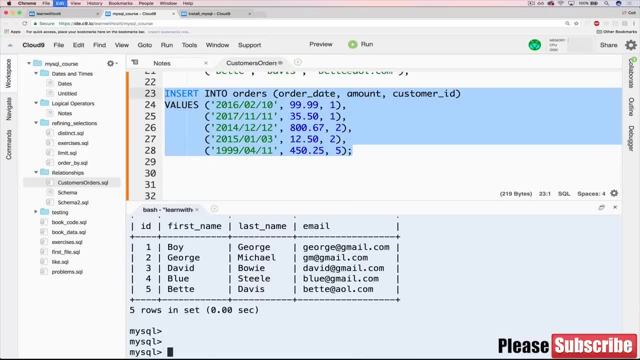 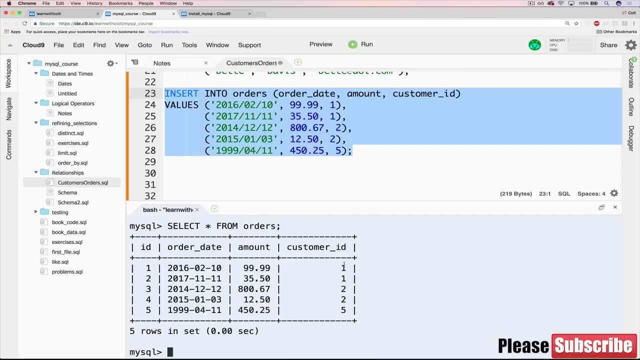 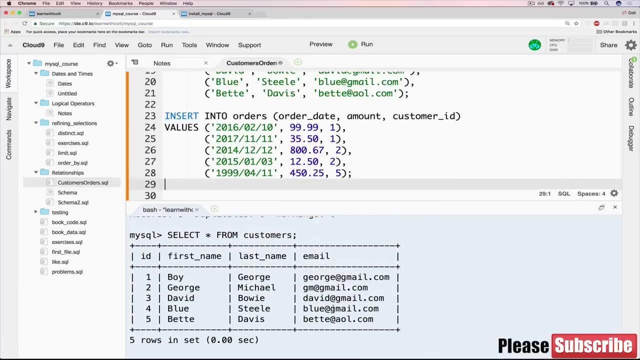 just going to do that now by copying this and pasting it in. And now, if I do a select star from orders, you can see we have customers Customer IDs 1, 1,, 2,, 2, and 5, which is fine. That looks good to us because we also have users who go up. 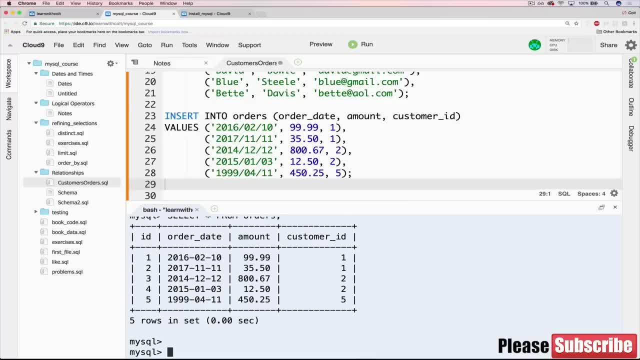 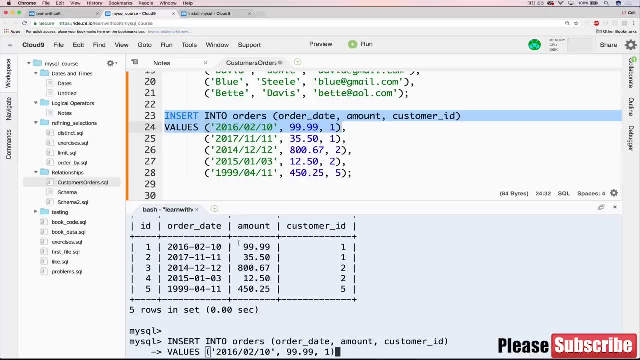 until 5.. But there's nothing stopping me from doing something like this. Let me just copy this first part. There's nothing stopping me from inserting something with, let's say, price is 33.66 or 67. Why not? And 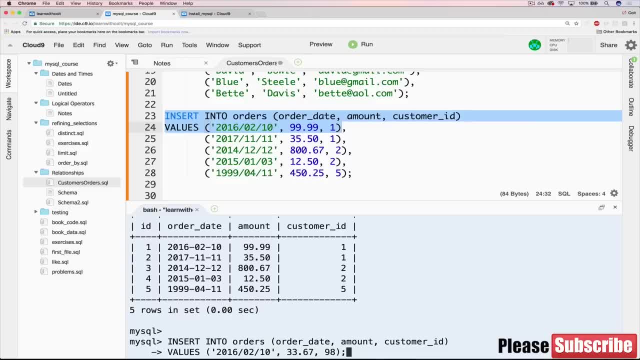 customer ID is 1, 1,, 2,, 2, and 5. Customer ID is 95 or 98. There's nothing stopping me from doing this, And that's not well. I mean, we could get by with this right. We could just know that we're never going to insert something with a. 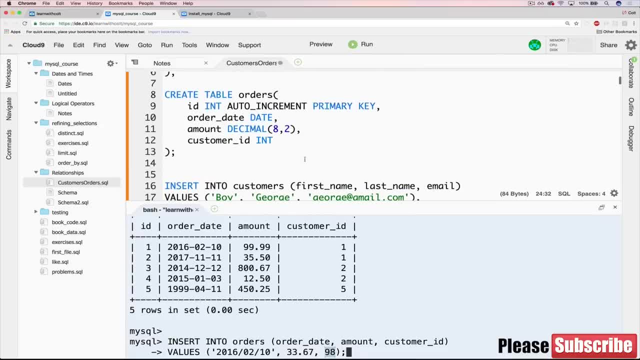 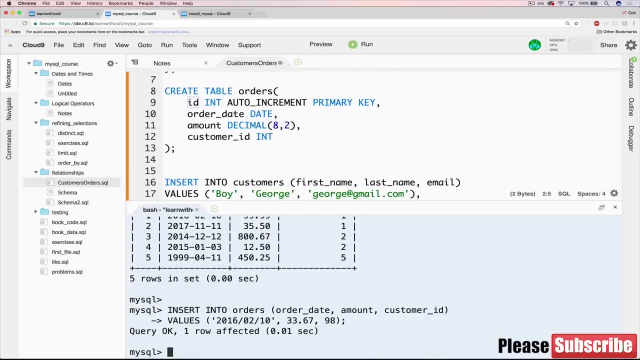 customer ID that doesn't exist. But because there is no association between customer ID and this ID, we can do whatever we want, which is usually not a good thing. So if I hit enter, now we have an order with a customer ID that doesn't exist. So I'm going to hit enter And now we have an order with a customer ID that 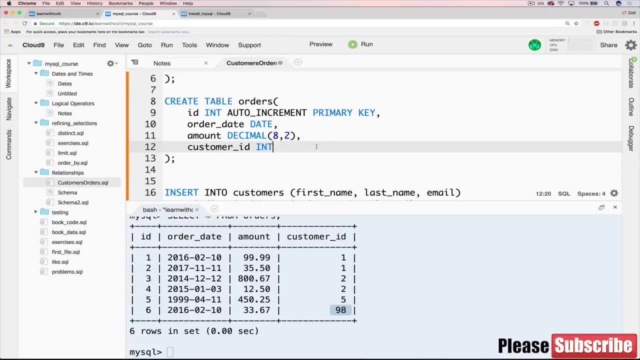 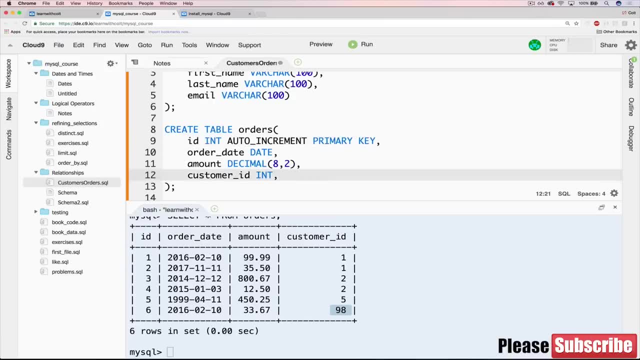 doesn't exist. So what we want to do is actually add in a constraint here. So, just like there's a primary key, we also can explicitly say: something is a foreign key. And the easiest way it's a little longer. It looks like this on a: 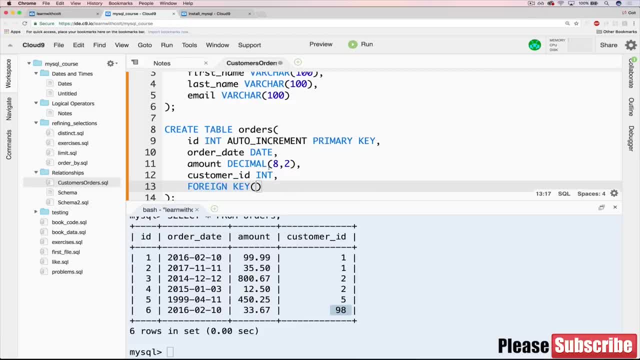 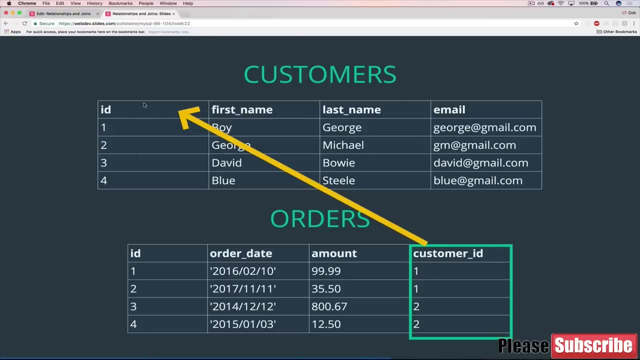 separate line, foreign key- and then in parentheses we'd say the name of the field or the column we're referring to, which is in the orders table- customer ID- And then we have to say what it's referencing. So it's referencing. think of drawing this line up to ID. Okay, so we have customer ID up there, So we're going to do. 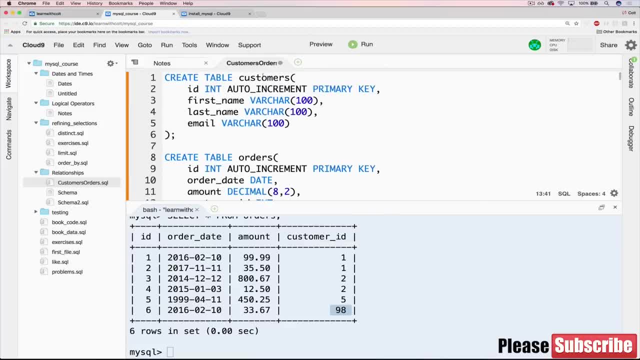 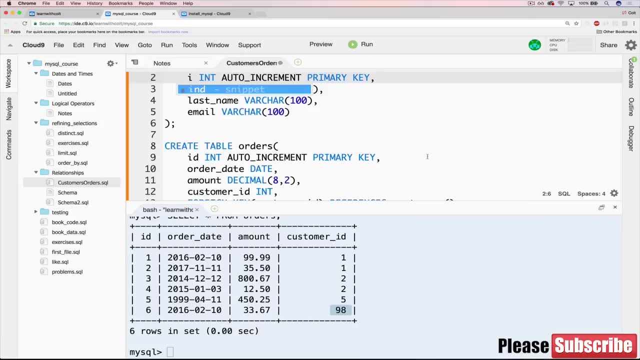 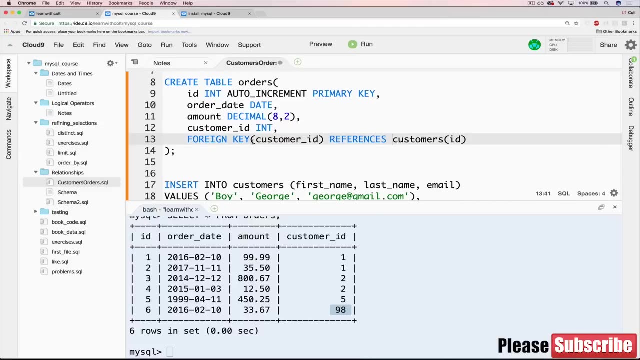 references, and then the name of the table, which is customers, And then, in parentheses, the name of the field, which is ID. Oops, I lost it. Here we are Okay, so it seems like a lot, But all that we're saying is: hey, there's this column. 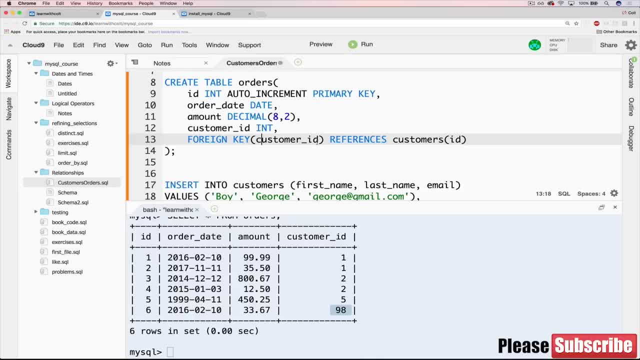 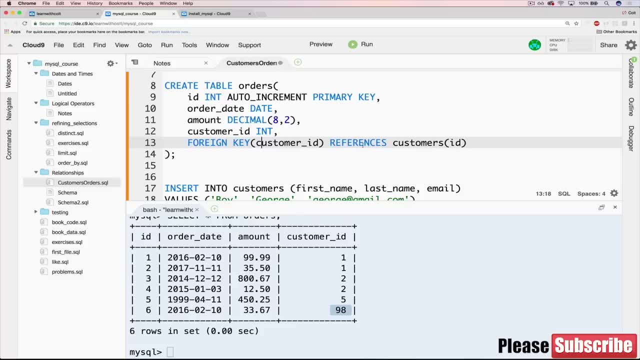 that we already defined customer ID. it's an int. Make that a foreign key And it needs to reference. remember, foreign key means that it's referencing something external, something outside the table. We want it to reference the customer's table and, in particular, the ID field. 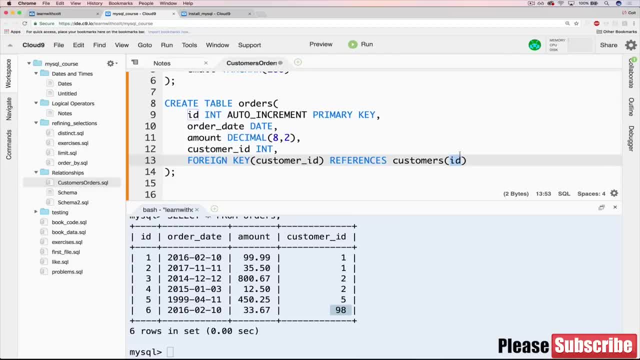 One small note I'll add. your keys don't always have to be IDs- They're almost always IDs- But you can get away with other things, Like I think we discussed this earlier. sometimes you want emails to be unique and you could make that a primary. 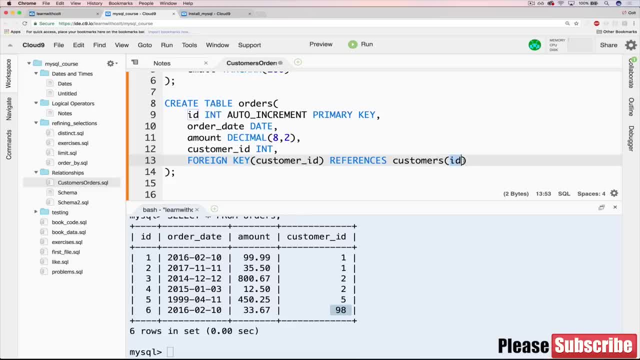 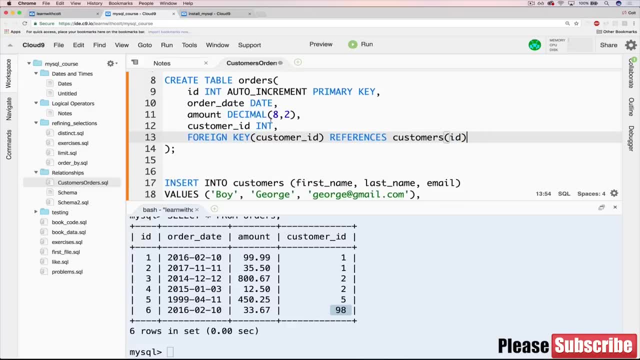 key instead. But IDs are easiest because they're short, They're simple, you can auto increment them and it's 99.9% of the time what you'll use. So here we go Again, just to go over the steps. 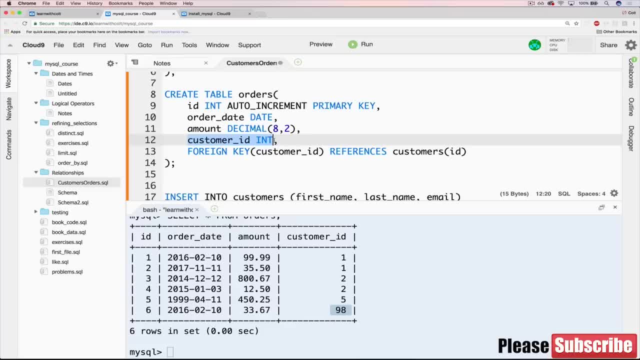 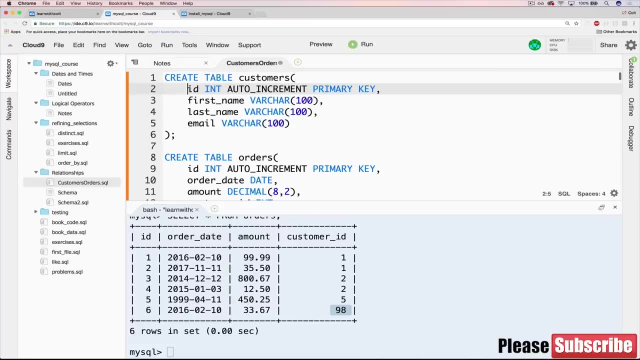 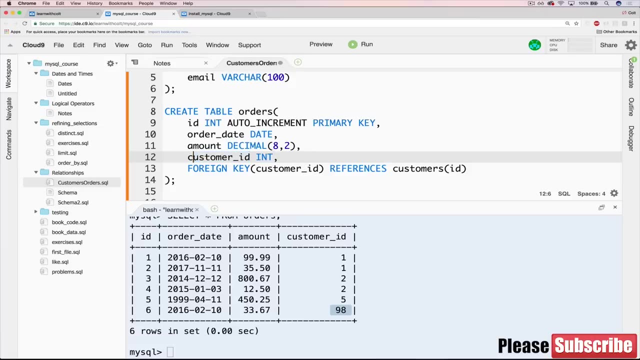 You define first customer ID And then, just to clarify, you can call this customer ID. you can call this whatever you want. I gave it just regular ID and gave this customer underscore ID, which is a convention when you have a foreign key to use the name of the table, underscore the name of the column. 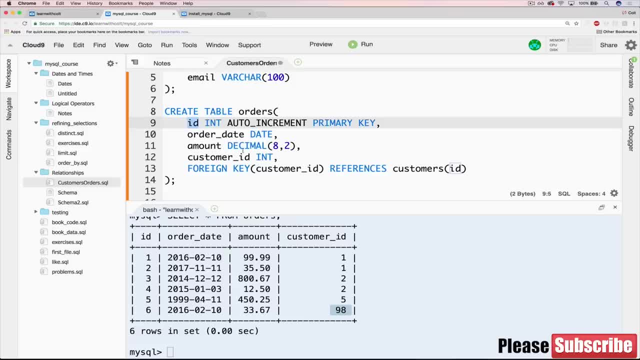 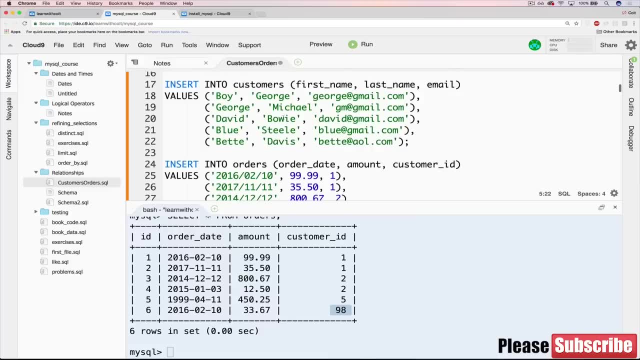 Just so that it's clear and you know we already have an ID here. Okay, so we're taking this, making it a foreign key, referencing this field here, So to see the effect of that, we're actually going to need to drop our tables and start over. 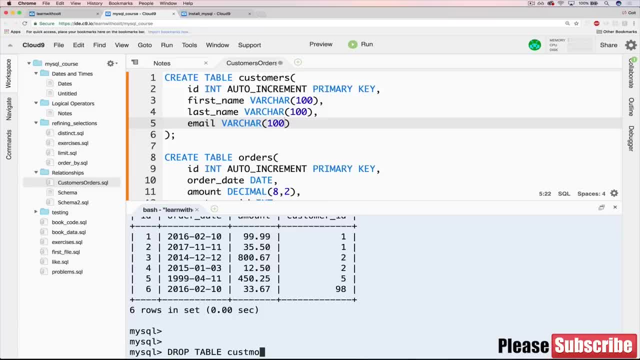 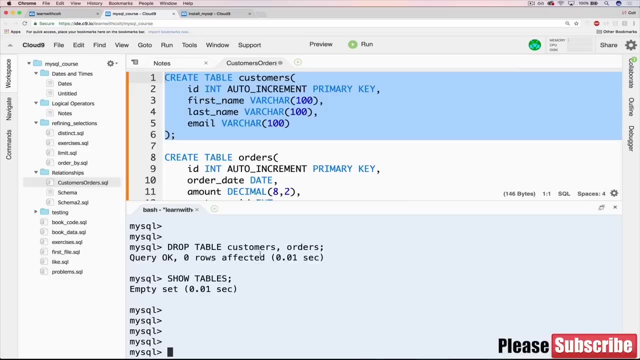 So it's just drop table and we can do them both at once. So customers orders, Okay, And now how do we see our tables? It's a quick review as well. Show tables, Nothing Okay, so I'm just going to paste this in again. We got our first table. 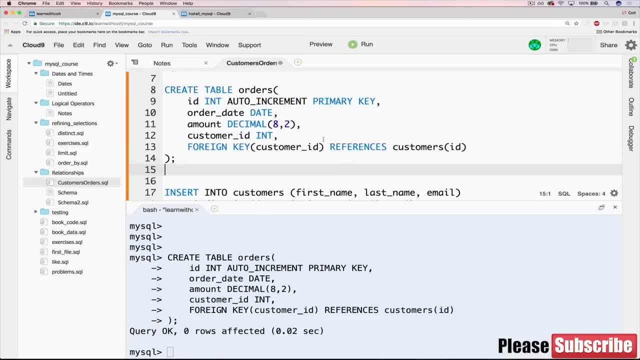 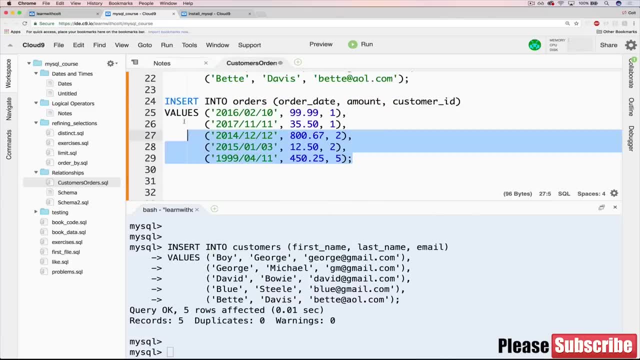 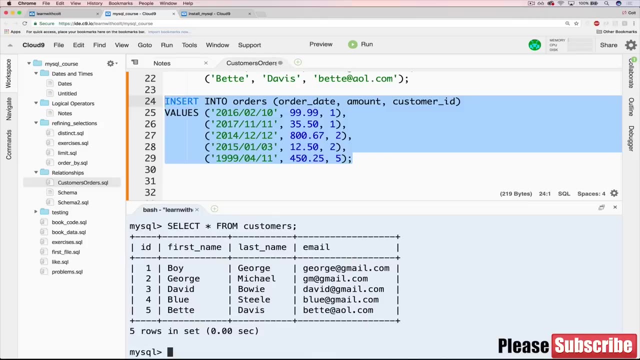 Make sure we didn't screw up our syntax at the second one Great. Only difference is this line here: Now we're going to insert our customers again And insert our orders again, And if we do a select star from customers, you can see nothing changed. 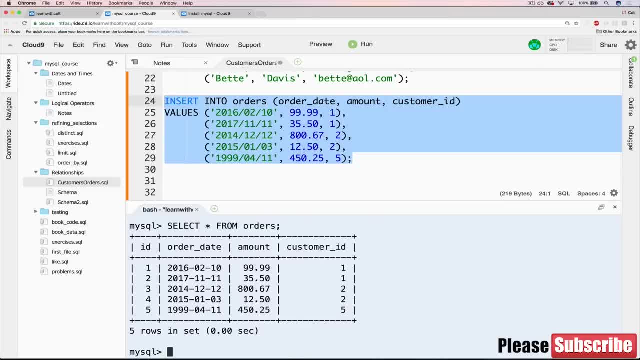 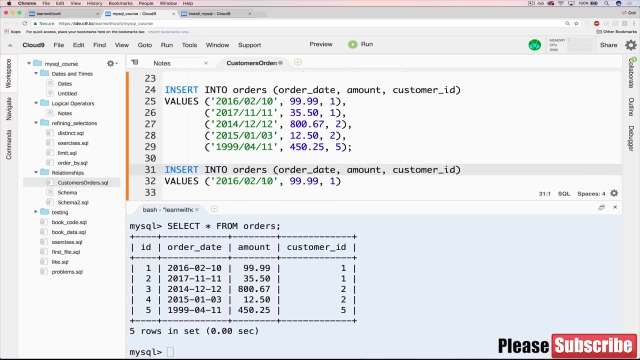 Do a select star from orders. Nothing changed, Great. But then now let's try and insert something else, Like what we did earlier. So I'm just going to copy this line again down below And we're going to insert an order. We can keep the same date, Let's do. 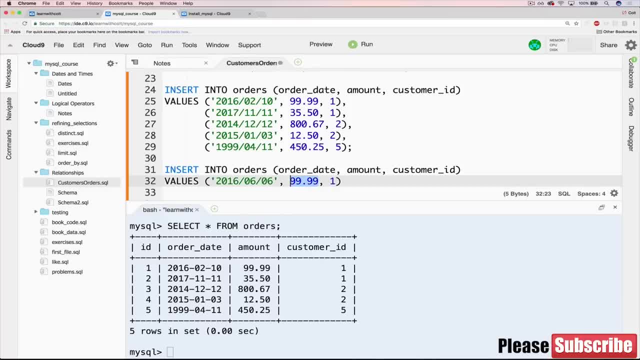 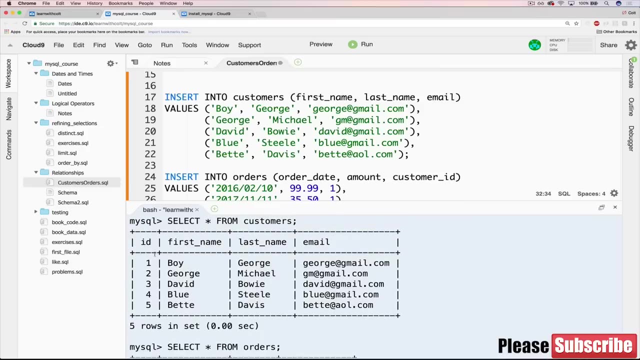 June 6th And our price will be 33.67.. But our ID is going to be 98,, which doesn't exist. Our customer ID is 98,, which doesn't exist as a corresponding user or customer ID. as you can see, We only go up until 5.. So if we 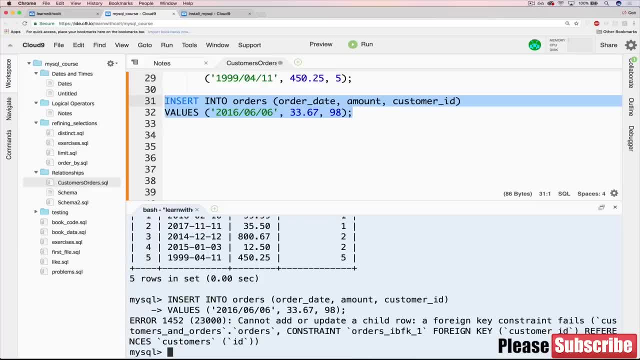 try that. now we have a problem which we didn't have before: Cannot add or update a child row. A foreign key constraint fails, And so basically it's saying I can't do that because the constraint you had said this was a. 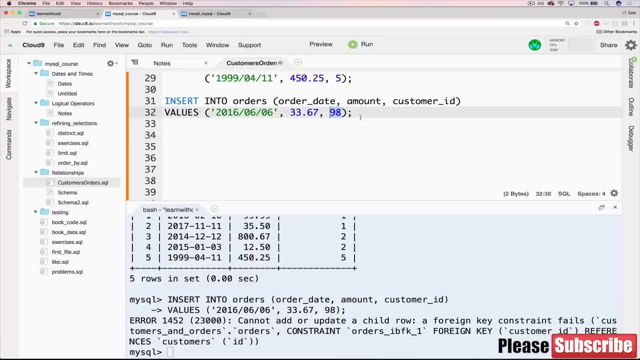 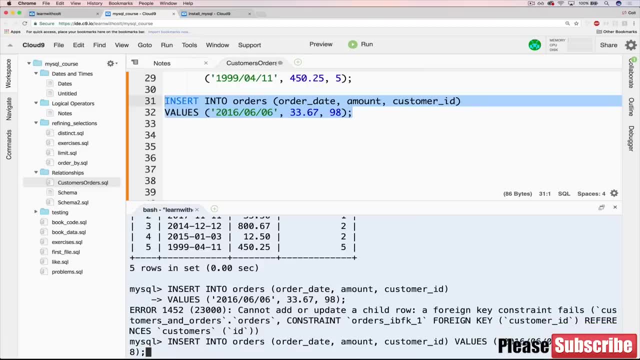 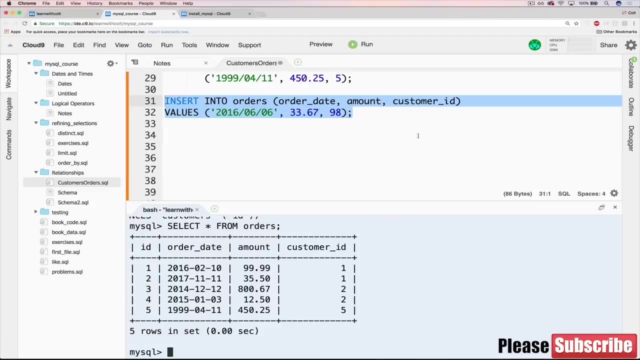 foreign key referencing customer ID or customers in the ID field, And there is no customer with ID 98. So it's now enforcing that, Which is great, And if we select all of our orders again, you can see it's not in here. It didn't make it in here, So we now 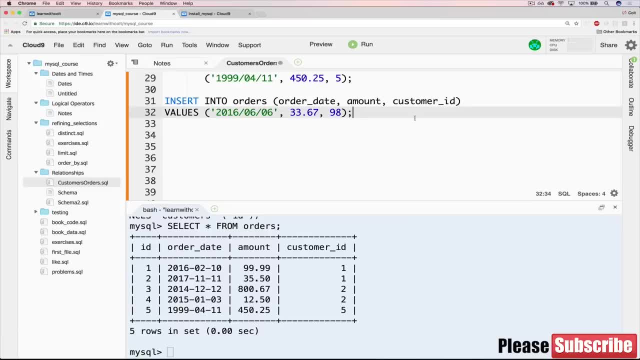 have this. think of it as a bouncer at the door that is checking if there's a corresponding customer, Which is useful. Okay, so that's what foreign key does, And I'll go ahead and end this video there, But we haven't really explored our data yet, So in the next video we're going to 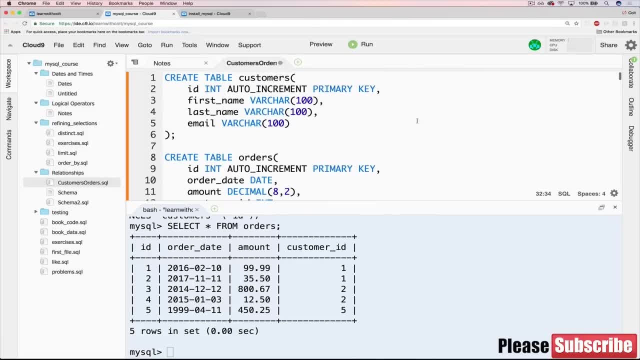 start seeing how we can work with our data. How do we basically connect these two tables? We have them associated, but now how do I do things with them? How do I figure out who ordered what Like? if I look at orders right now, 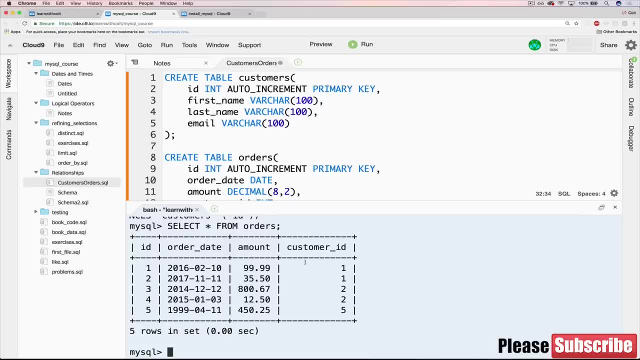 I have a customer ID, But what if I want the name of the person, The first name, Or both first and last name, Or the email? So that's coming up in the next video And we're going to dive into a really important topic, which is joins. So that's coming up. 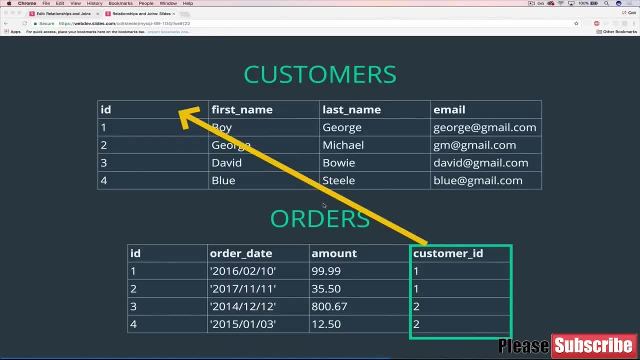 Okay, so we've got this data in our database. We have two separate tables that are distinct. They have a foreign key, The orders has a foreign key referencing customer ID. But so far we haven't actually done any queries, We haven't worked with our data. So let's try it now. 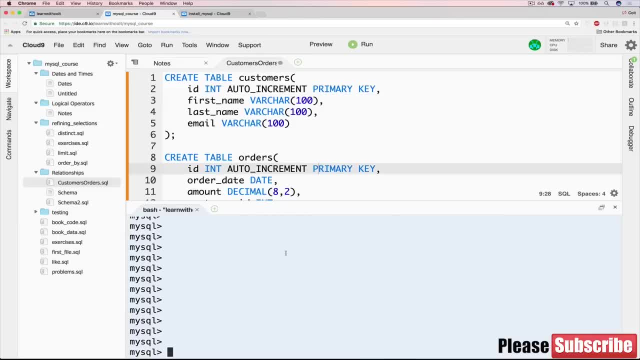 So back over in Cloud9.. Let's start with a simple question. Let's look at our customers. Well, actually let's look at our orders, And I have five different orders here. Let's say, I want to find the orders that have been. 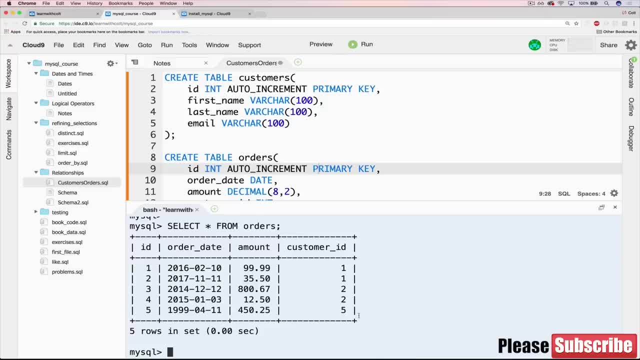 placed by Boy George. So how do I do that? I want the orders placed by Boy George. Well, we could do it as a two-step process. So I would first say basically: find the customer, find the ID of the customer whose. 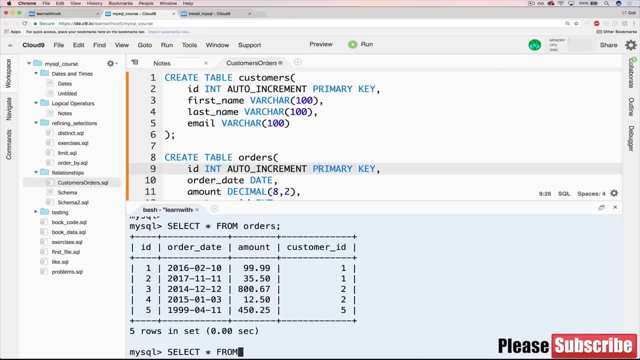 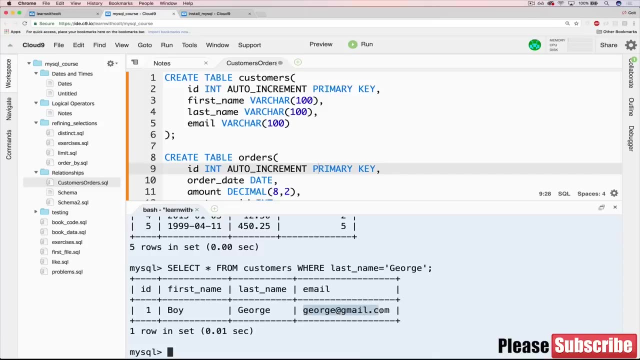 name is Boy George, So we could do select star from customers where, And then we would do something like where last name equals George. Okay, so we get Boy George George at gmailcom And his email- excuse me, his ID- is 1.. Okay, so then we take that and we go to. 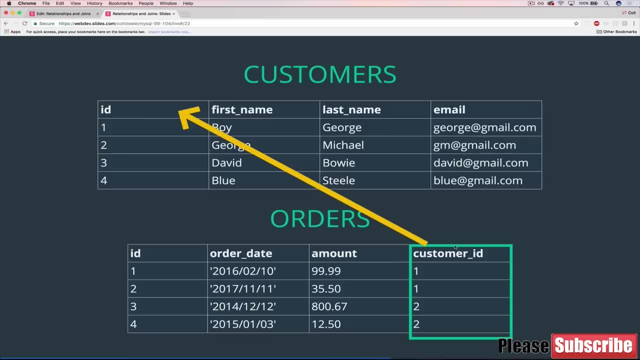 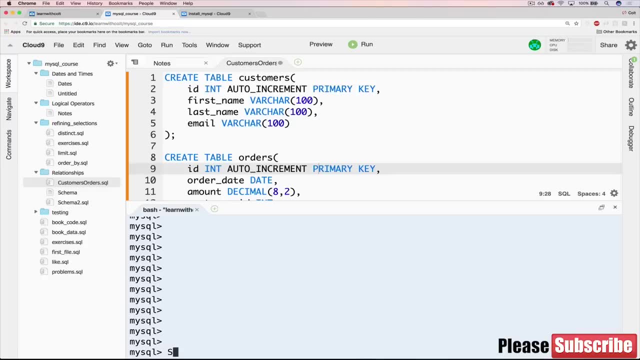 our orders table And we try and find: okay, where is in the orders table, is customer ID referencing 1? So we're just going to do a select star from customers where- excuse me, select star from orders- where customer ID equals 1.. 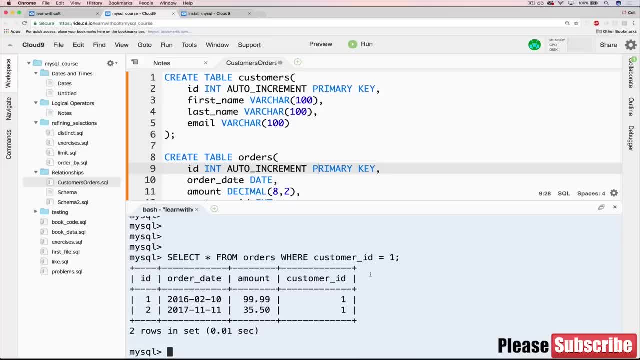 And there we go. These are the two orders placed by Boy George, So that was a two-step process And we could simplify that, Or we could at least do it all at once, Actually, using something that we touched on. We could use a subquery, If you'd like to try and do that. 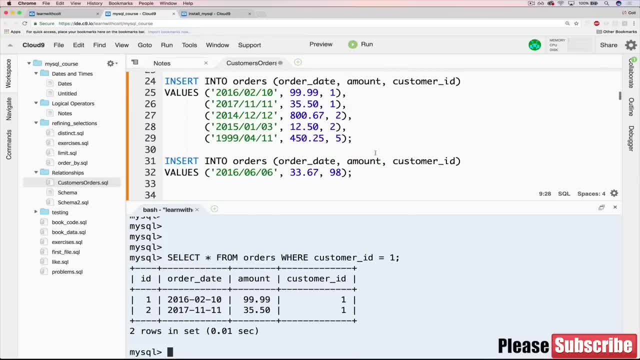 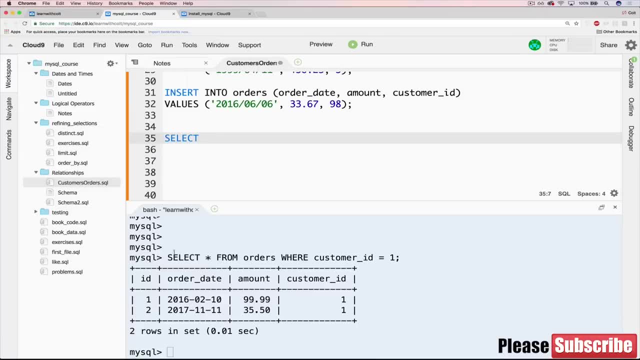 you can take a moment to figure that out, But I'm just going to write it down here. We would do something like this. So the two things we just did, Let's just copy this one. We did this right here. Select star from orders where. 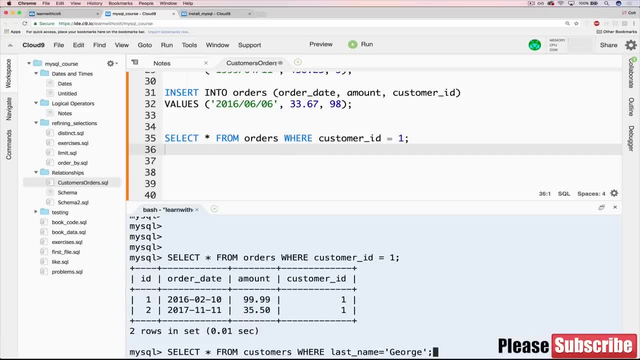 customer ID is 1.. And then we also had select star from customers. So to put them together, what we basically want to do is find the ID of the customer where last name is George, Then plug that into here, So rather than hard coding it as 1.. 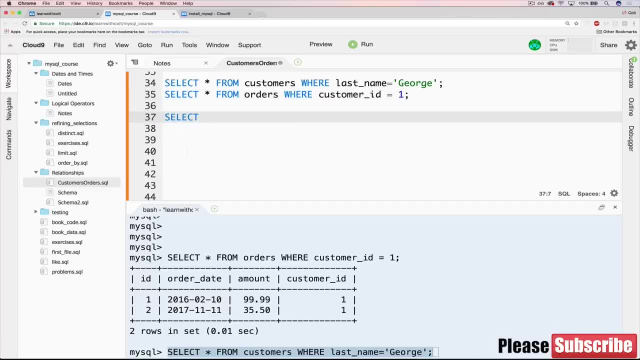 So it would look. it's going to be a bit long. It's going to be something like select star from orders where And then where is going to be long. So it's going to be a subquery And we want to do where. 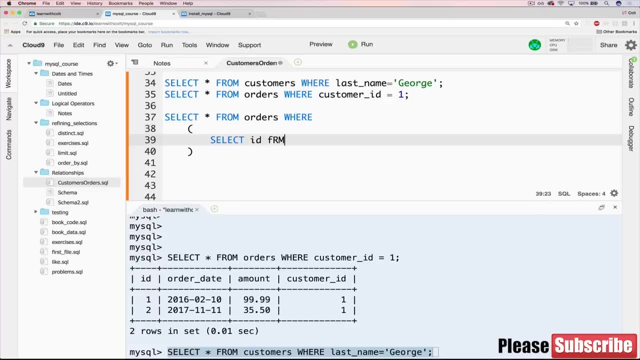 select ID from customers where last name equals George. Okay, So let's take a look. We need to fix one thing: actually Select star from orders where customer ID equals the result of this. Okay, So let's step through it. Start with this middle part. This runs, It selects. 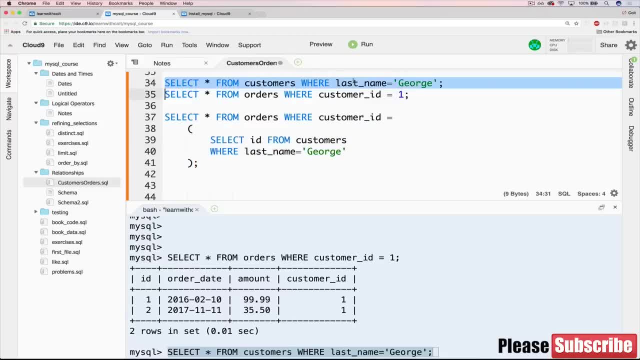 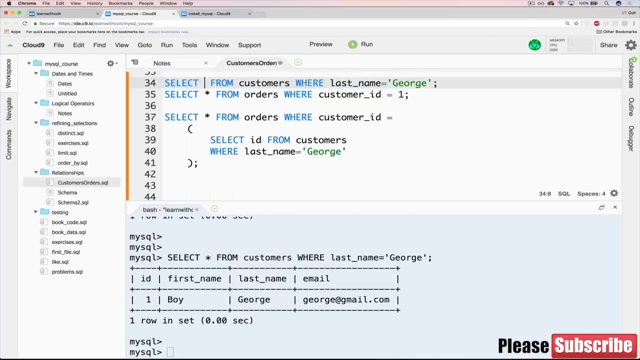 ID from customers where last name is George, Which is what we did up here. So when we run that, we're only selecting ID. So actually we could change that, Because we're only selecting ID And it gives us 1.. So you could think of: this whole thing is replaced with 1.. Actually it's more like 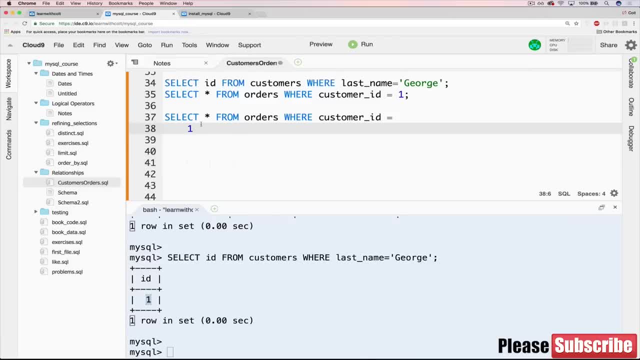 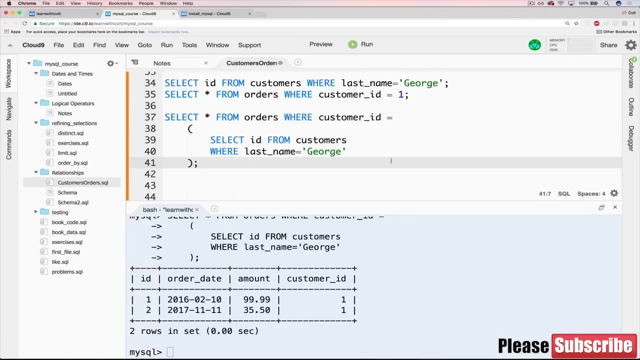 this whole thing is replaced with 1. Which leaves us with select star from orders where customer ID equals 1.. So let's test it out And you can see we get the same result. But this is still not ideal. It's a bit cumbersome, And this is only. 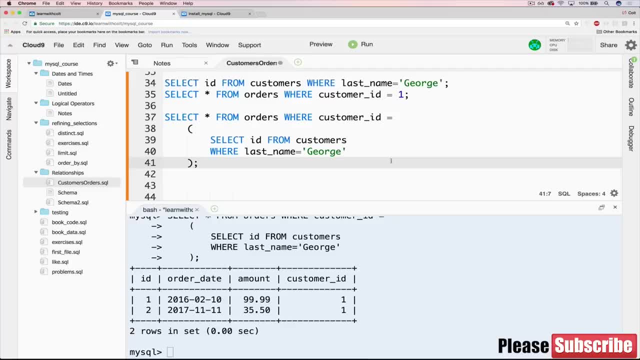 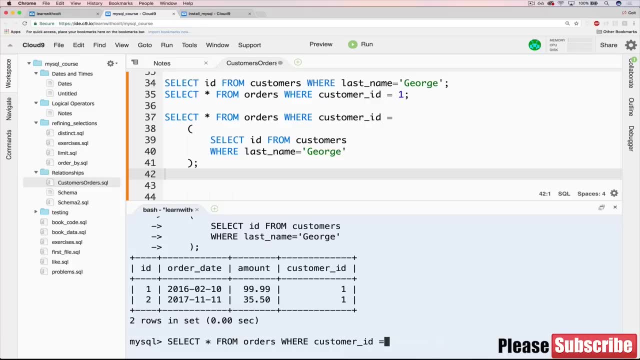 if we're working with one user anyways. What if I wanted to see a synthesis of my data, If I wanted to see next to every order? So something like this: If I go up, Let's do select star from orders Next to every order I wanted. 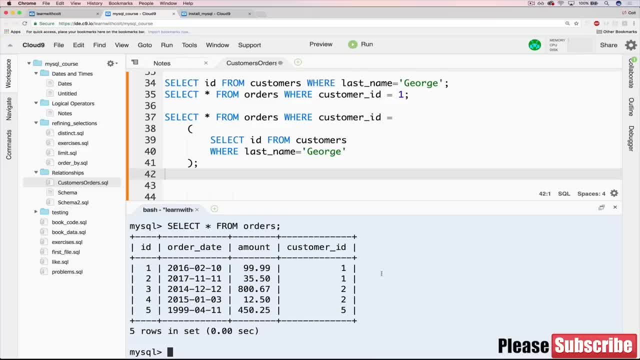 it not just to say customer ID, I wanted it to say the name of who made the order. So Boy George, George Michael Betty Davis, And I wanted that to be printed here. So how do we do that? And this leads us to our next topic. 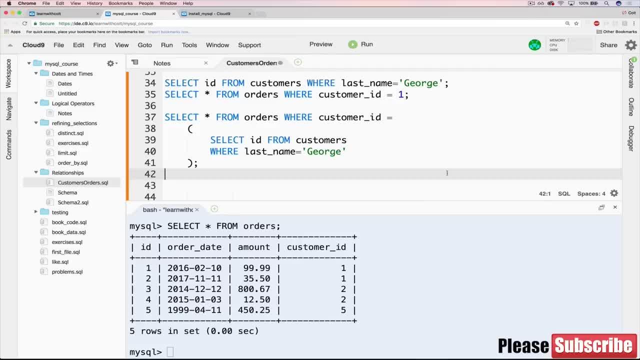 Which is joins. So joins, allow us to accomplish that. The whole point of joins, Which is sort of this buzz, wordy, maybe intimidating, mysterious thing to some of you, The whole point of it is that it takes two tables And we can conjoin them in a couple different. 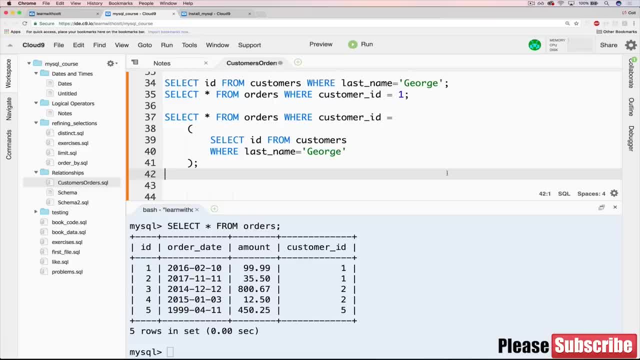 configurations, So we'll talk about what those are. That's the next few videos, But we can conjoin them Basically take the data from one and take the data from another and stick them together In usually a meaningful way. But I'm going to show you one way that is not meaningful. to start, 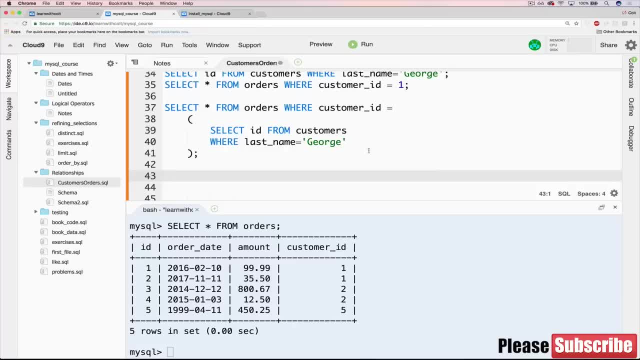 And this will be our first, most basic join that you probably will never use. I never have used it, But it's good to know And it just looks like this. Select star from orders. We can do customers first, It doesn't matter. 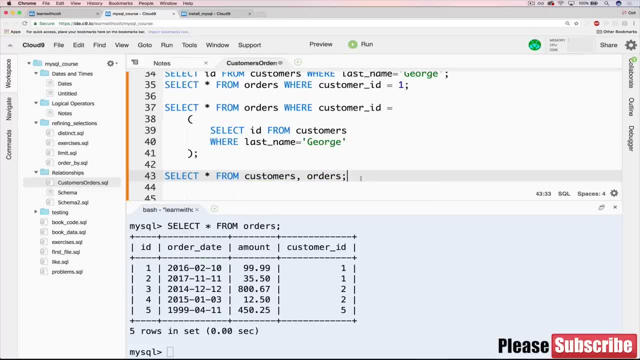 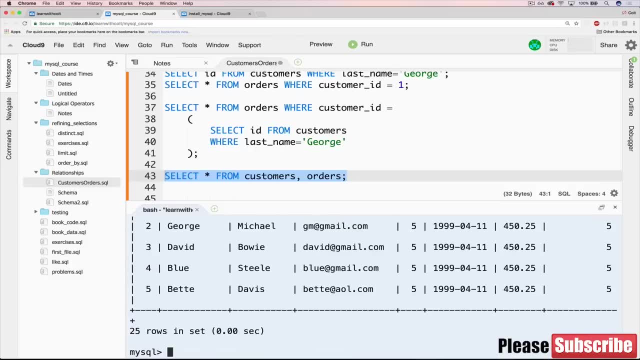 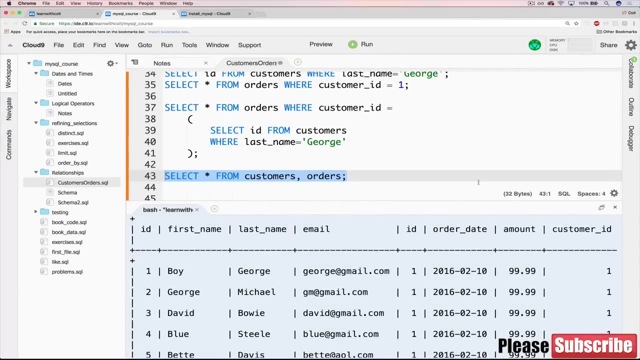 Customers, comma orders, And that's it. So if we just select from both of them, What do you think will happen? I'm going to hit enter here And we get this monstrosity. It's very long And what we're actually looking at is called a cross join. 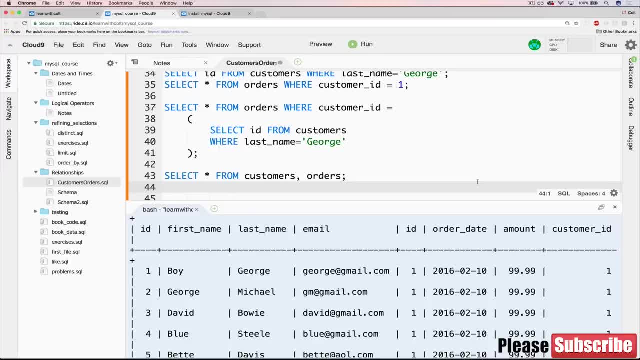 I think I've also heard it called a Cartesian join. Like I said, it's pretty useless, But it's interesting to see. What it does is it takes every customer. So we have Boy George, George Michael, David Bowie, Blue Steel, Betty Davis. 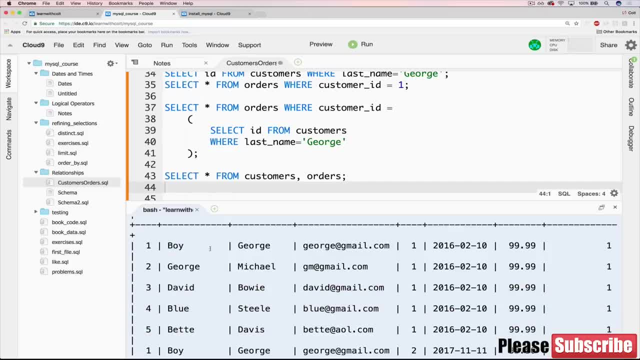 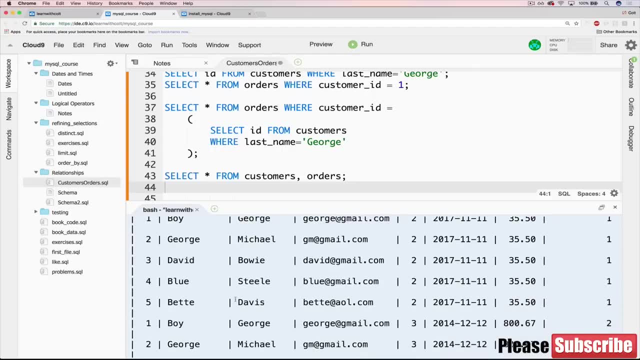 But then notice that let's ignore the right half, Just the customers. It goes from one to five And then it repeats: Boy George, David Bowie, Blue Steel, Betty Davis, And then Boy George, George Michael, David Bowie, And it keeps going. 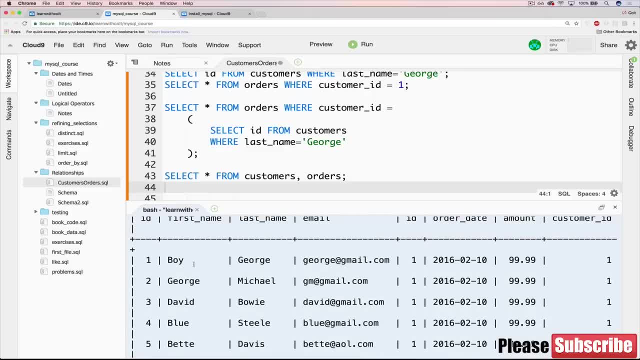 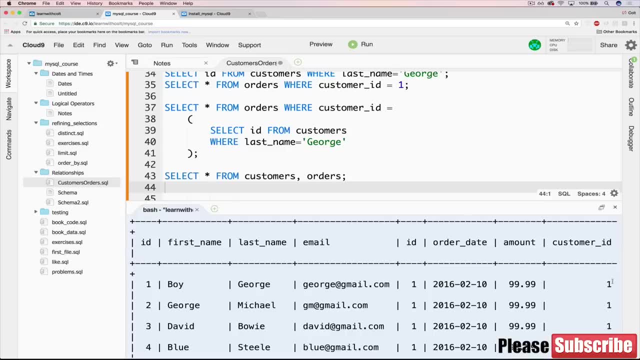 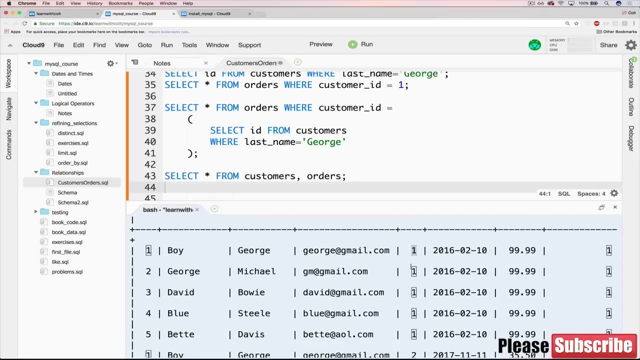 And what it's doing is taking every customer and conjoining it with every order. Think of it as almost multiplying them. So it's taking the first order, which is $99, with an order ID of 1.. And it's sticking that next to. 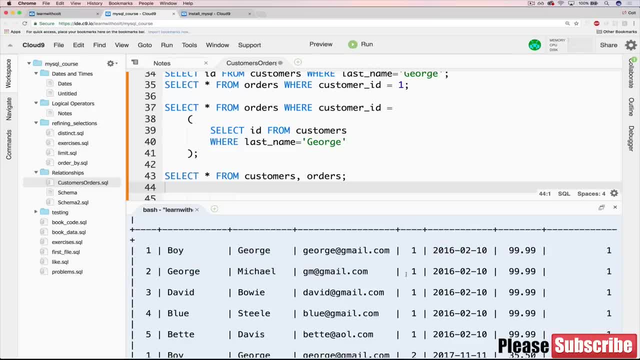 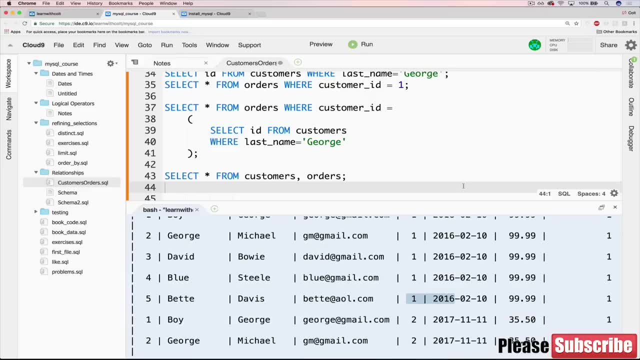 Boy George order ID 1.. George Michael order ID 1. David Bowie: same order. Blue Steel: same order. Betty Davis: same order. And then it moves on to the next order. So then we go back. Boy George stuck with. 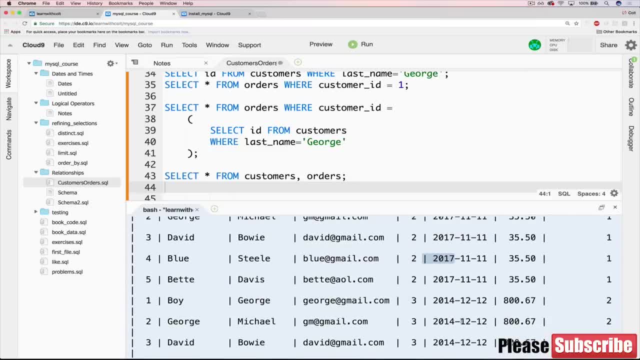 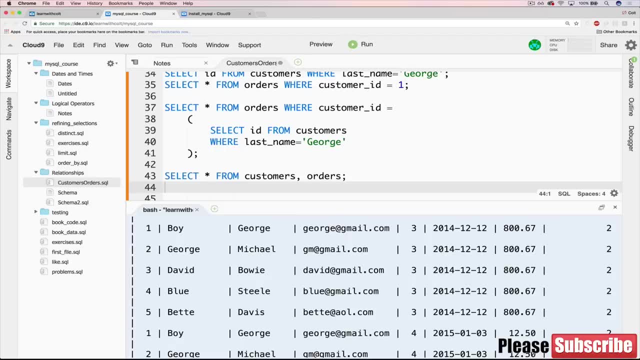 the second order. Second order. second order: Basically. hopefully you can see what's happening. It's a lot of text to look at, But it's taking these two tables and just jamming every row, every possible combination, next to each other. 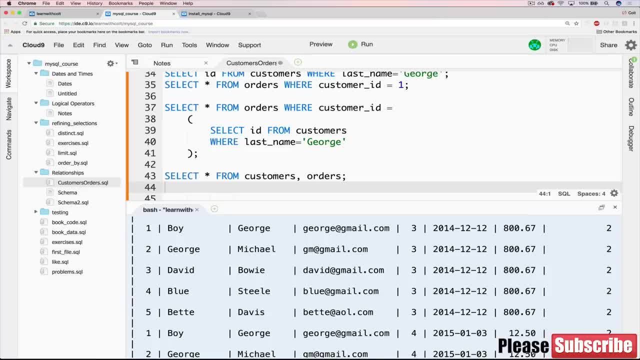 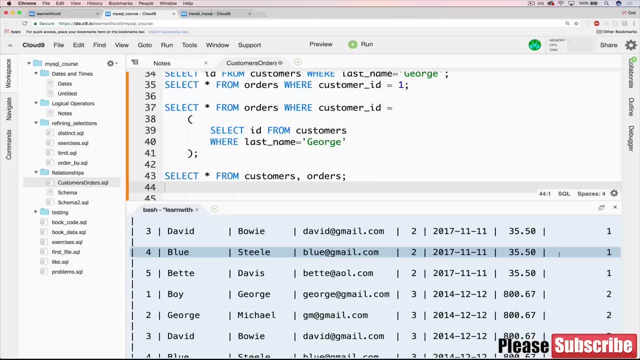 Which is meaningless. There's no reason to do it, But I just wanted to show you it because it's the first and most basic type of join, So don't make much of the fact that you can do it. It's just good to know that you can. 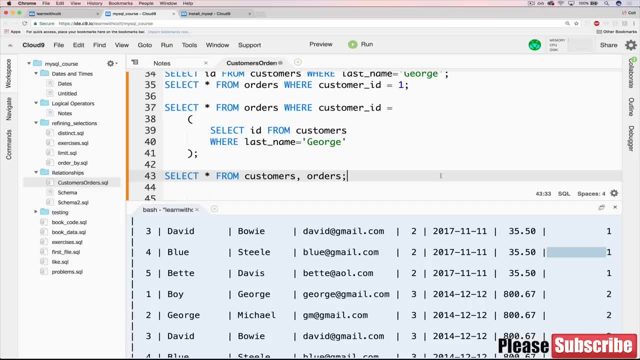 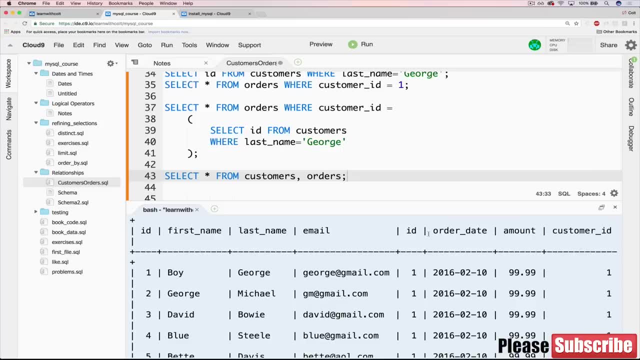 But we're much more interested in basically whittling this down to the stuff that we care about. So maybe the most obvious and meaningful way would be to whittle it down so that we only see where there's actually overlap, So where the ID of the customer is the same. 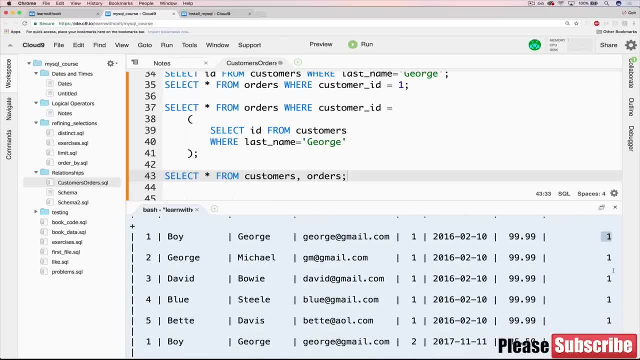 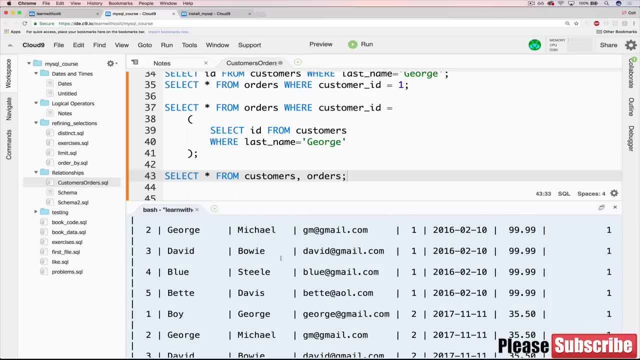 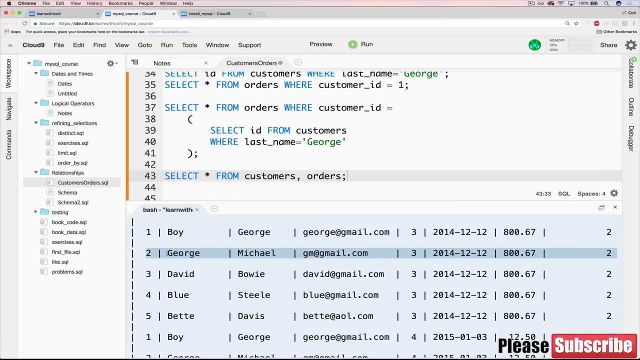 as the customer ID. So this would be a match right? This is an order placed by Boy George, But then none of these are actually placed by the customer they're next to. But then we get down here and we have: okay, here's George Michael with an ID of 2. And he placed this order. 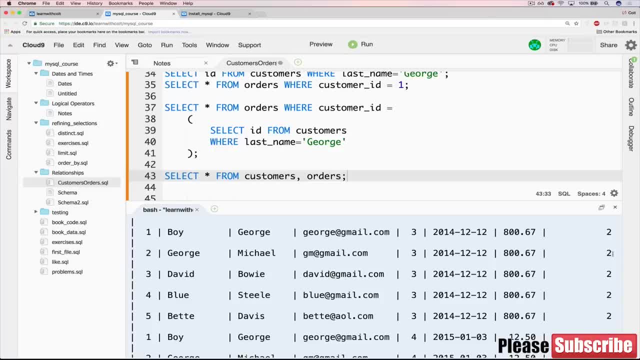 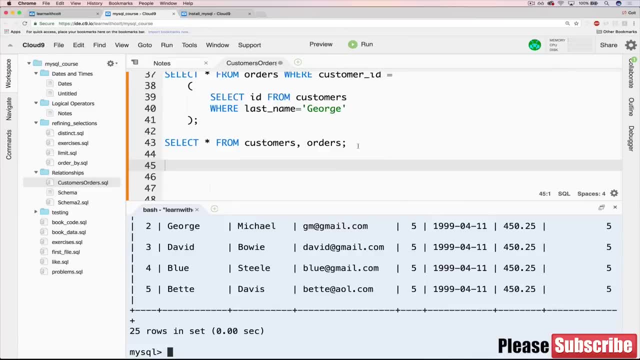 So how do we whittle it down to that? And that's what we'll see in the next video. Sorry for the cliffhanger, Okay, so in the last video we saw our first join, our first example, which is actually something. 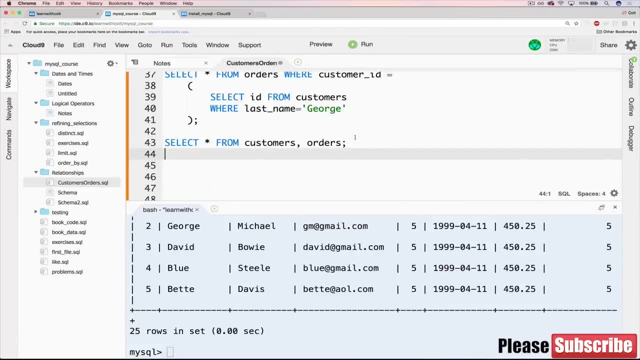 known as an implicit join, which you'll see for a moment why it's called implicit And it's also, in particular it is a cross join, Useless. basically, Think of it as multiplying our data, cross multiplying. It takes every. 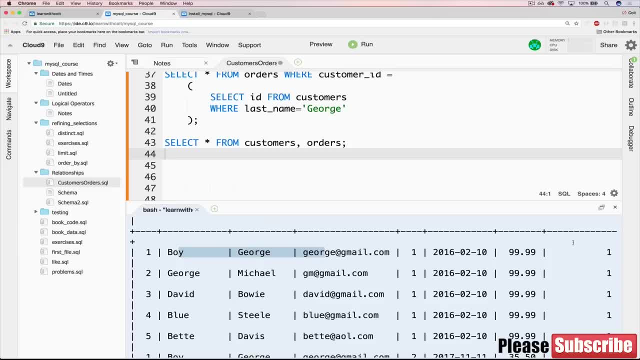 possible combination. So we have Boy George. Well, I don't need to go over that again, I'll bore you to death. So now we want to focus on whittling it down to what's actually relevant. I want to see the name of. 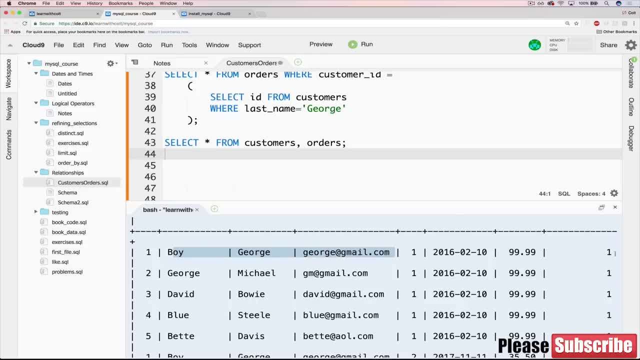 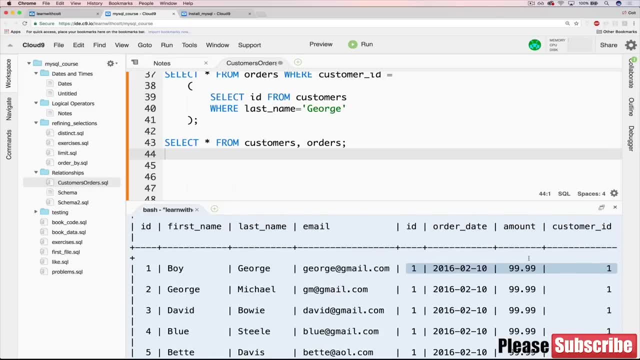 the name, first name, last name and email of every user who actually placed an order next to that order, Not just every arbitrary order. I want the ones that they placed, And so we're getting sort of close If we have all of it next to each other. now we just want to. 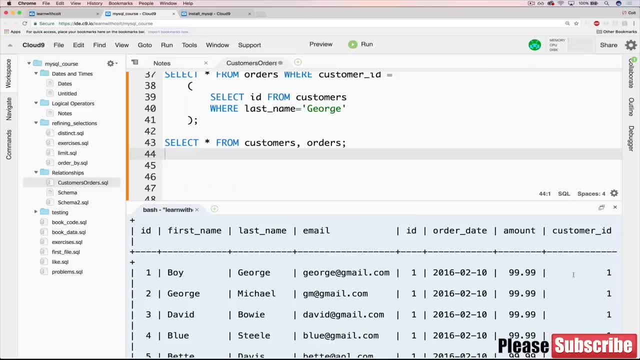 only select the rows where, what, What condition is true, Where our user ID is equal to the order customer ID. So it's just like any other kind of select we've done, where we just can add in a where, So it will be a select star from customers comma. 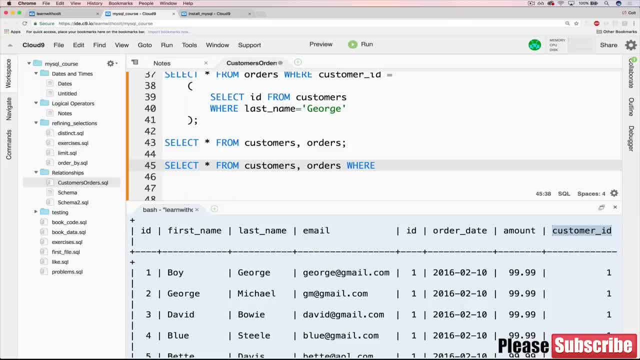 orders, where and where. what is true? Where ID from the customer is equal to customer ID. So we could do this where customer equals customer underscore ID. But there's a problem. Maybe you've identified it. We have two IDs. Remember, we're just taking the customers table and the orders table. 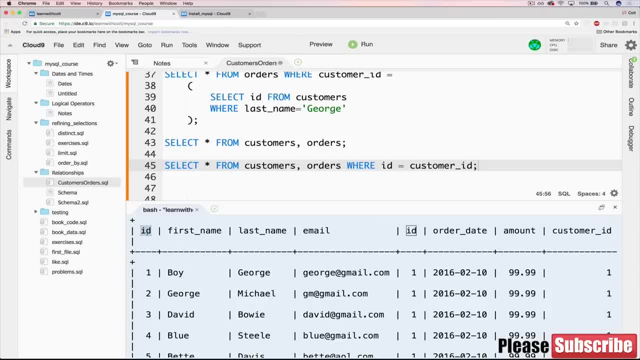 and putting them together. So we have ID from customers and ID from orders. So what does this refer to? That's a problem. Fortunately, there's a work around. It's very, very simple. All we have to do is prepend the name of the tables. So this should be. 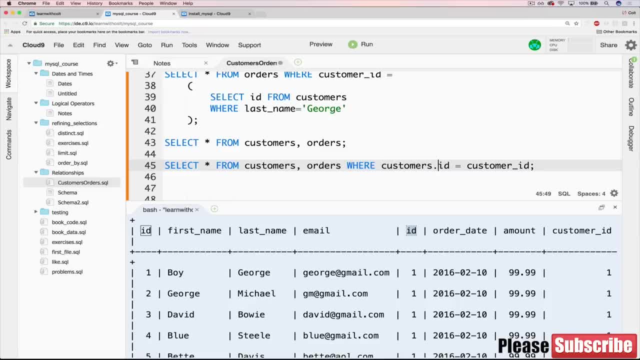 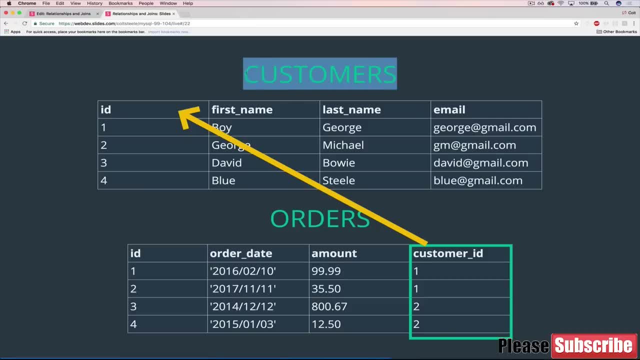 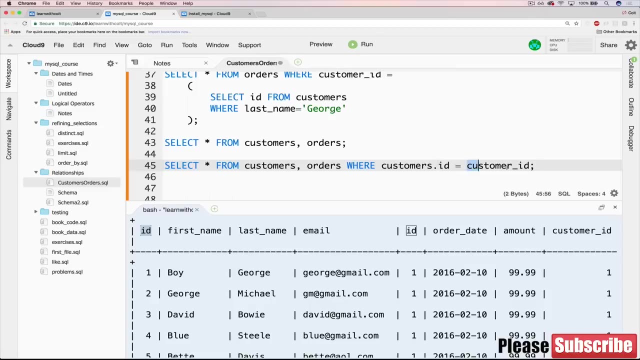 our customers ID. right, It's coming from here And just to make that clear what's happening, We're saying where the customers table dot ID, So where this is equal to customer ID, Now customer underscore ID, And I realize there's a lot. 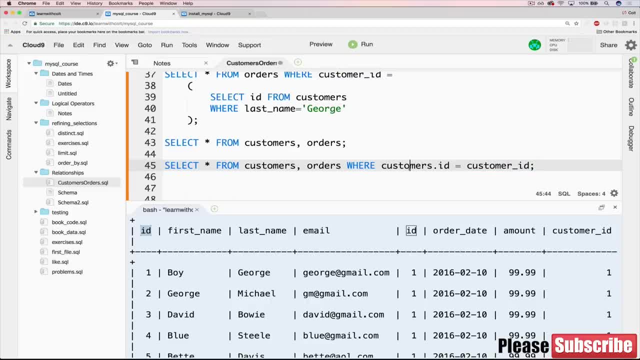 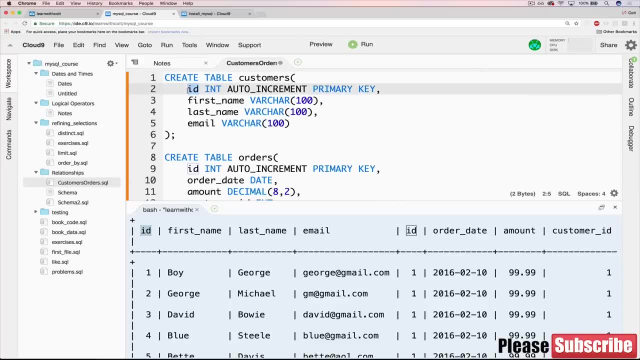 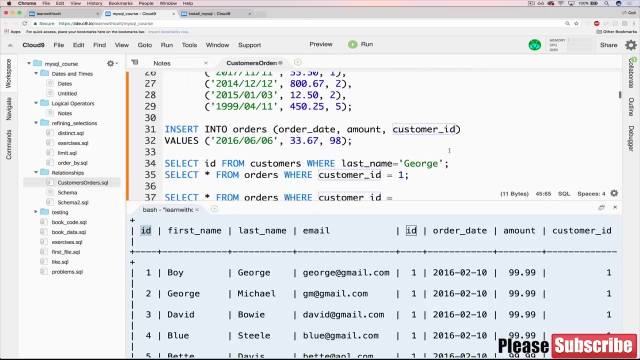 of saying customer and ID over and over, But these are different Right. This is the customers table ID. It's referring to this Customers dot ID. That dot means in the customers table And this is customer underscore ID, Which is referring to this right here. 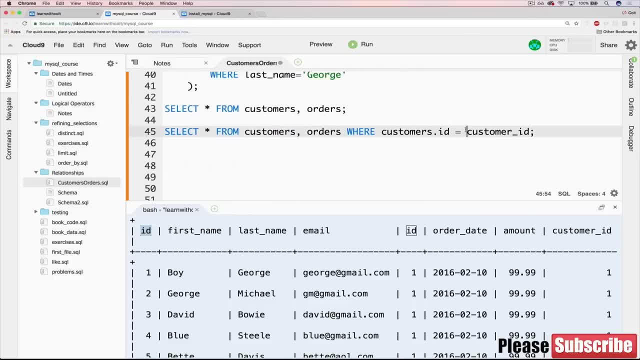 So we don't have to say orders dot, customer ID. But it's a good convention to follow to do that. Just to, whenever you're working with two or more tables, to be explicit about which table or which row- excuse me, which column. 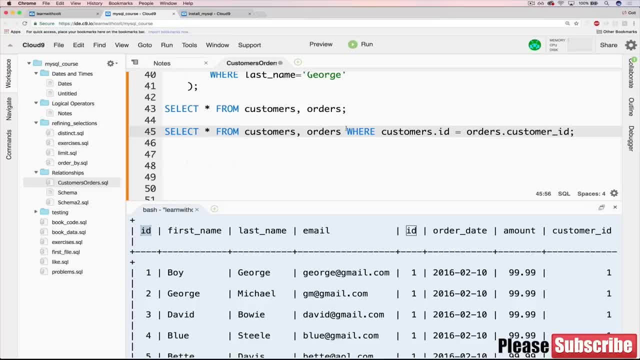 belongs to which table. Okay, So we have this line. Let's copy it over. So what this will do is select, or it's going to do this cross join, but only where the customers ID, customer table ID- is equal to the customer ID of the order. 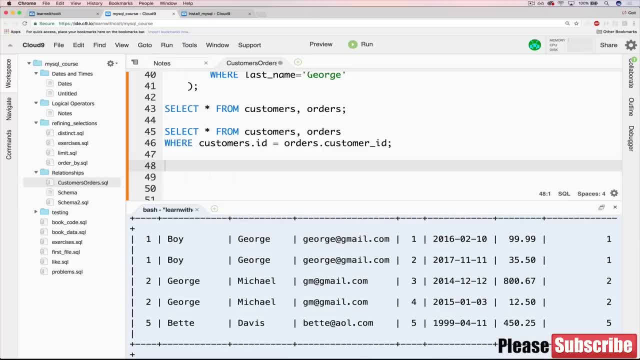 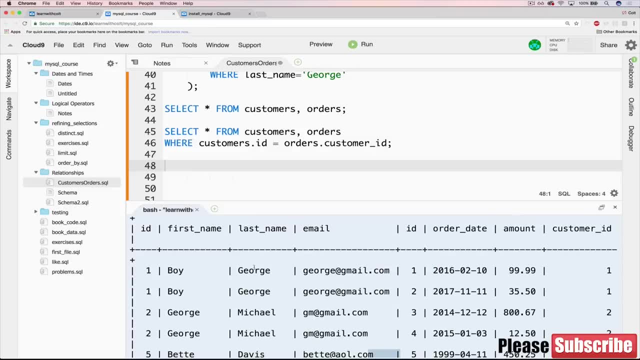 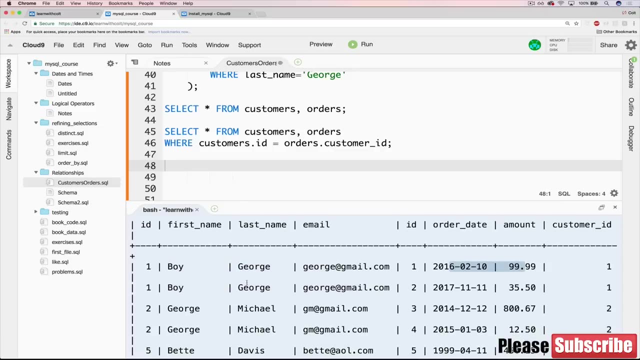 So now, if we do this, take a look at what we get. We have five orders, So we get these five different rows And we have the corresponding customer who placed it. So Boy George placed this order for $99.. Boy George placed another order for $35.. George. 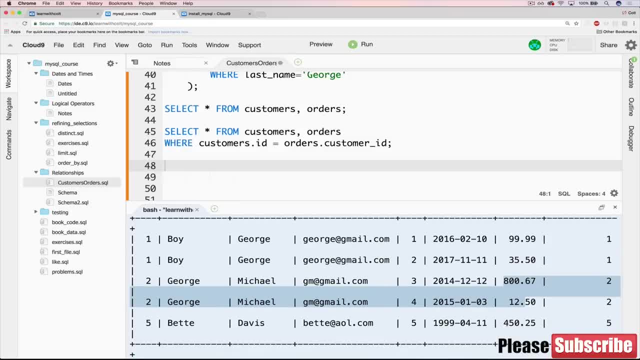 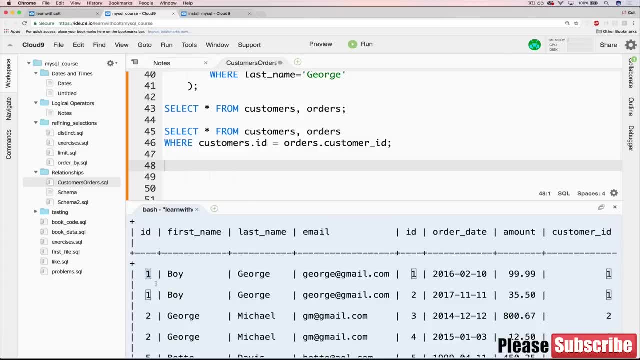 Michael placed these two orders And Betty Davis placed this one order for $450.. So you can see we have customer ID over here And it's matching the customer's ID And of course we could condense this a bit. So maybe we don't want star. 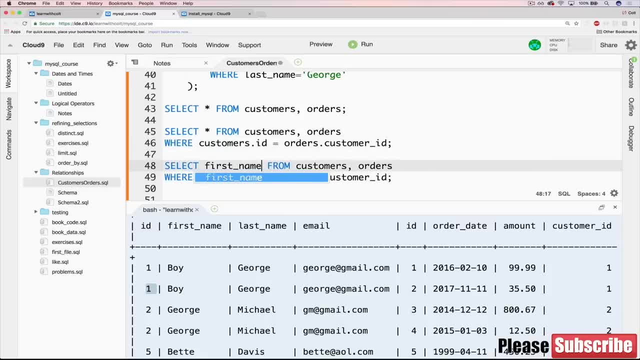 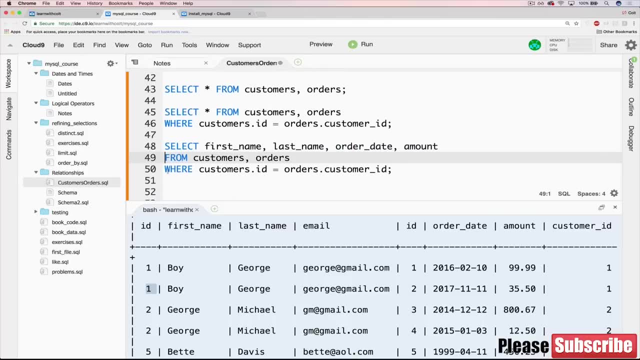 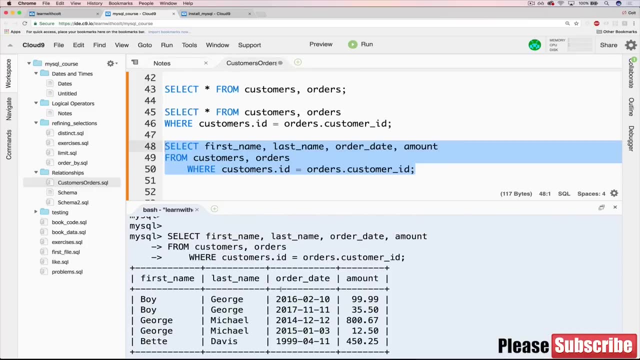 Maybe we want first name and last name And then order, date and amount, And that's it Just like that. So let's try it. And now we get a more condensed table that has that information. Boy George, Boy George. two orders: George Michael: one order. George Michael another. 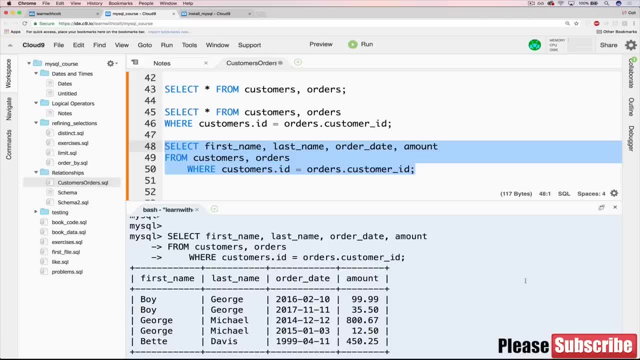 order. Betty Davis: another order. So what we've just done there, we have joined them together using what's known as an implicit inner join. So I'll write that here. Okay, And that's what we did up here as well. So, 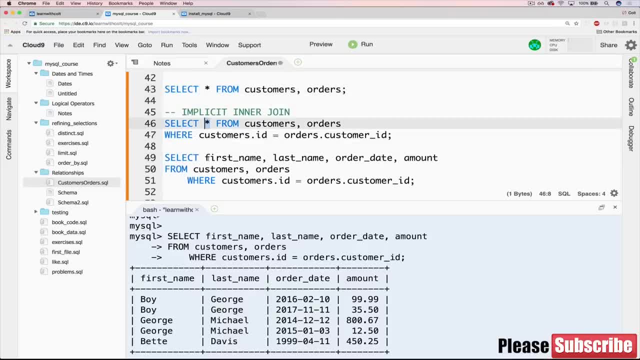 this is just a more refined one, because we're not selecting star, We're only selecting a couple of things, But we've joined them where they match, if that makes sense. So I have a simple diagram. It's very, very ugly, But a simple diagram to show you, And I'm sorry it's so ugly. 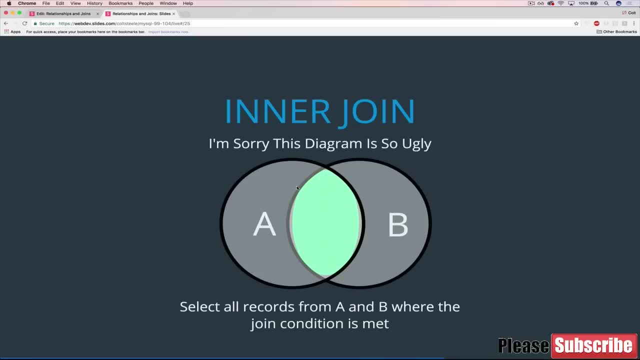 It was very difficult filling in this shape here. It's not a circle And the slides tool I used doesn't let you draw weird shapes. You have to do circles. So I'm sorry, I really am, But what's happening here is that we have two tables right: Customers and 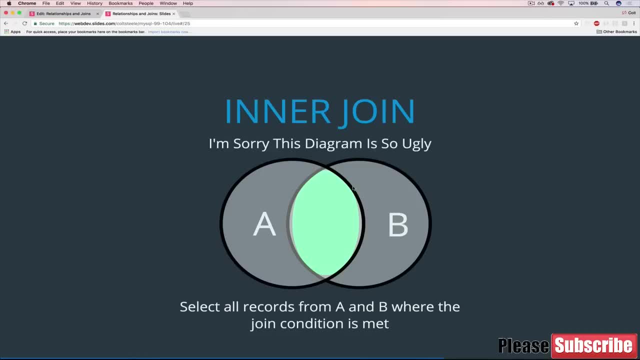 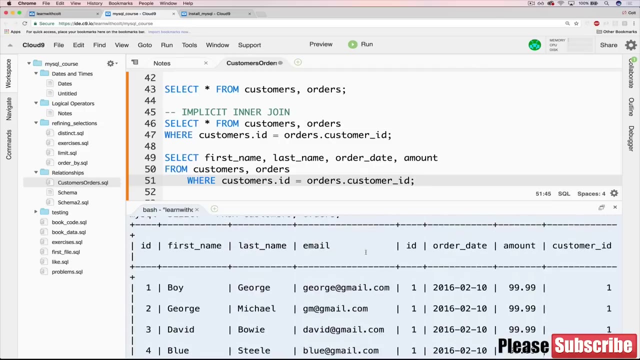 orders, And what we did at first was select everything, Combine them and just take everything together. But all that we want to do with an inner join is take the inside where they overlap, And that's what we did. We went from this monstrosity and we whittled it down. 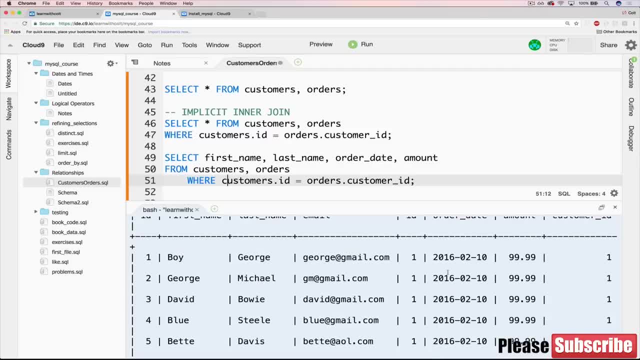 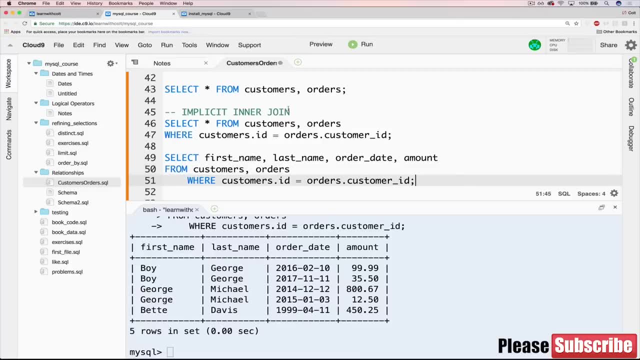 to where the customer's ID is equal to customer ID in the orders table And we get this right here. Okay, Now I said this is implicit And that's because there's an actual, explicit syntax. There's a better way of doing this, And when I say better way, I mean 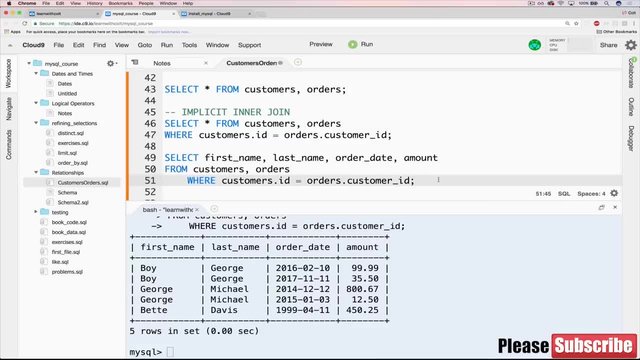 better. It really means that it's more conventional. If you're not familiar with that, it means that it's think of it as like an unwritten rule that developers follow. They think it's cleaner. It's more easily understood to do it this way, which I'm about. 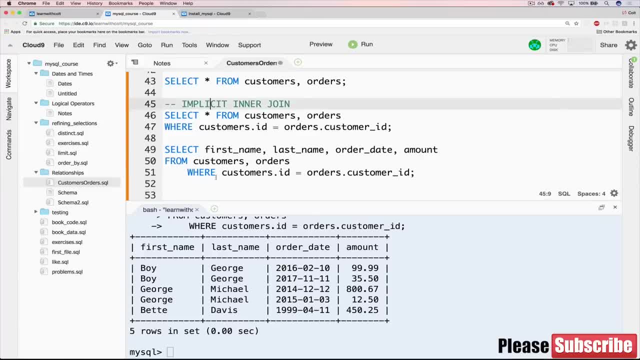 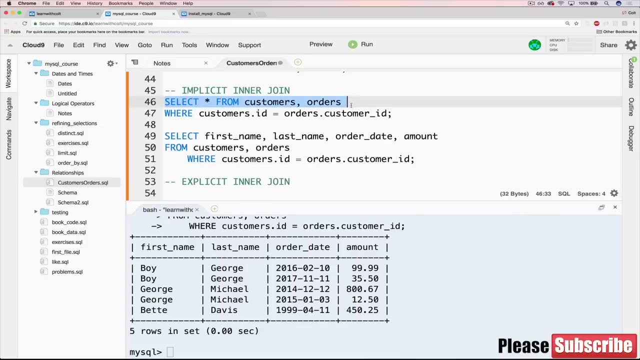 to show you. So I'm going to write: ooh, what did I do? Here we go. I'm going to write: comment: explicit: inner join. And this will be the first time we see a new keyword called join. So we're going to do our same: select star. we'll start with this. 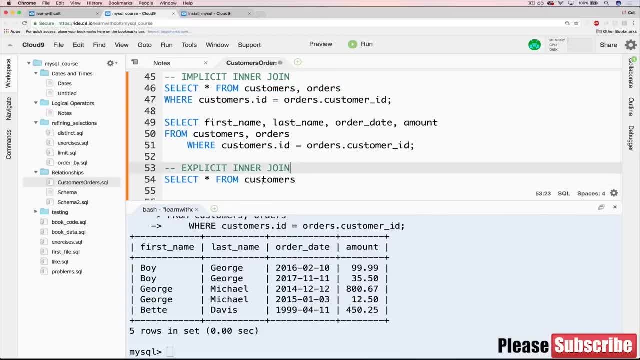 one from customers. However, we're not just going to do comma orders, We're going to select star from customers and then we're going to add join orders. So we have some new syntax. I'm just going to type it all first And then we're going. 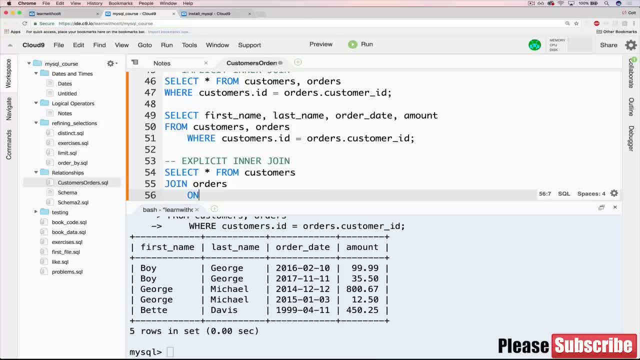 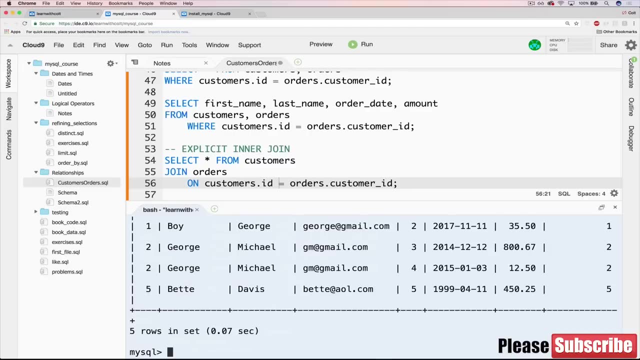 to tell it where We're going to join on. customersid equals orderscustomerid. Okay, So if I copy this and I run this, it does the exact same thing And, if we want to, of course we could refine this more. 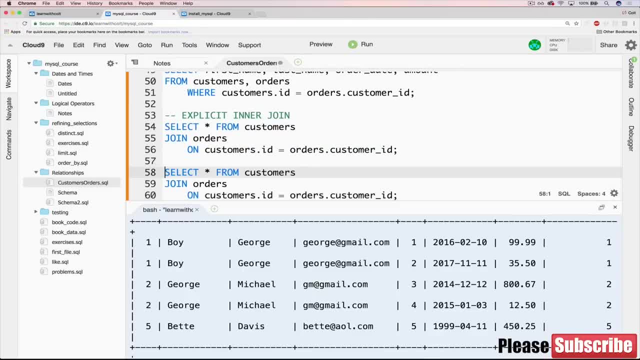 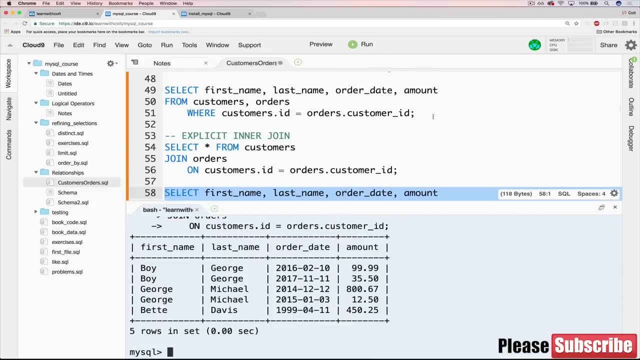 just like we did earlier. So instead of selecting star, let's do the same thing where we select first name, last name, order date and amount. Okay, Copy this over, And now we get this same table, just to prove to you that it's the same. 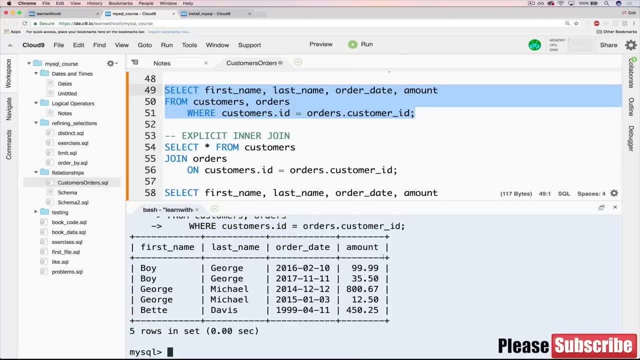 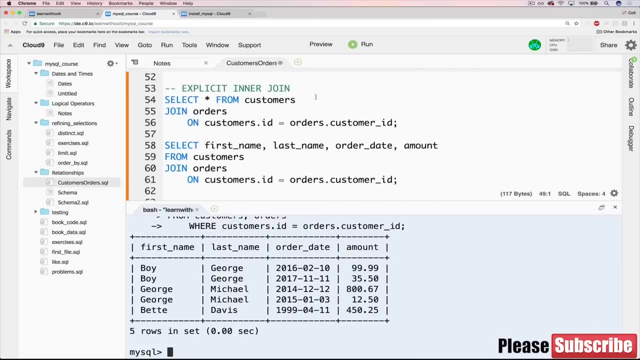 There you go. Can't even see a difference when I just hit enter And it looks like the same thing is here. Okay, So this is still an inner join, but this time it's explicit. and it's really only explicit because we're writing the word join. So when we say join order, so we say: 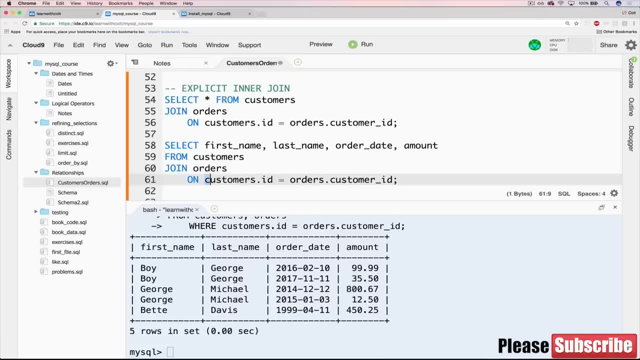 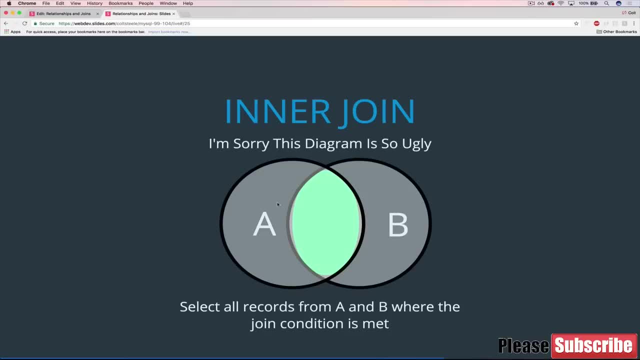 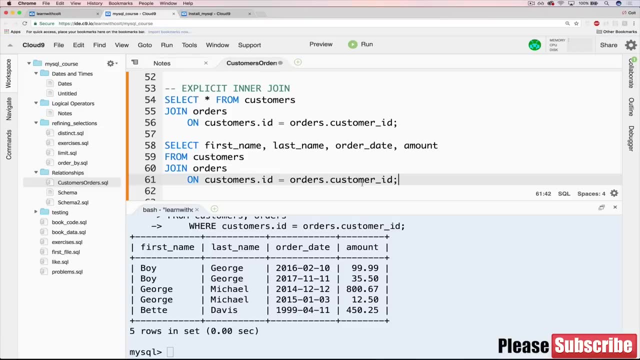 from customers, join orders on this join condition. So take the left and the right, so customers and orders, these two circles basically, and join them. create the union table where customersid is equal to orderscustomerid, So where the id from here matches the customer id from here. 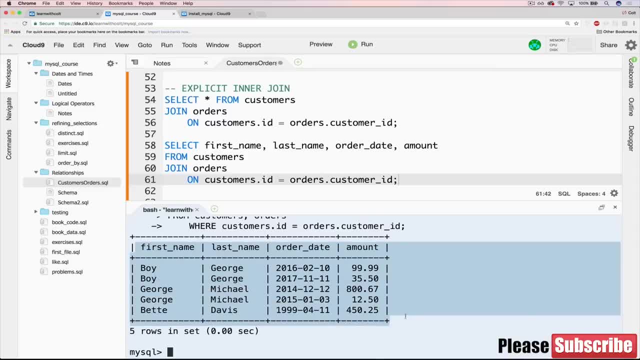 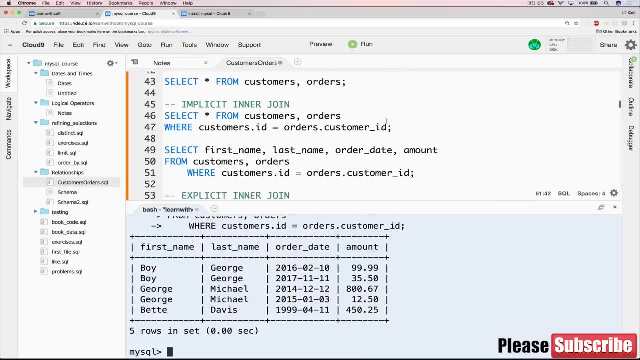 take that overlap and make this table for us. So I know it's a lot that I'm talking about here: The term inner join and explicit inner join, implicit inner join, and we're going to next talk about right joins and left joins. 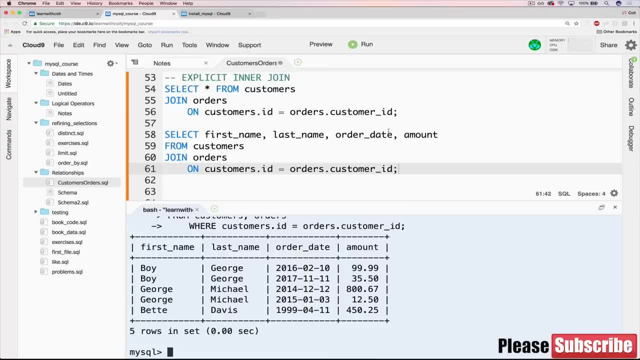 It can't be overwhelming. So all I want you to focus on is the key idea here: that we are joining data together based off of a condition- Right, And we could join it off of some meaningless condition too, just to show you. So if we go, 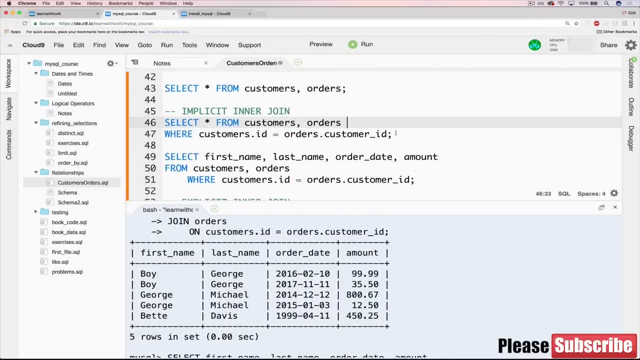 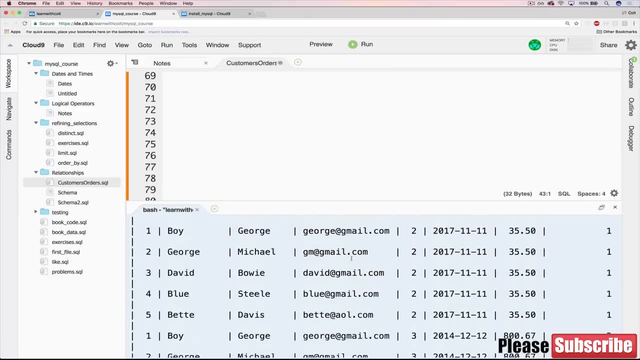 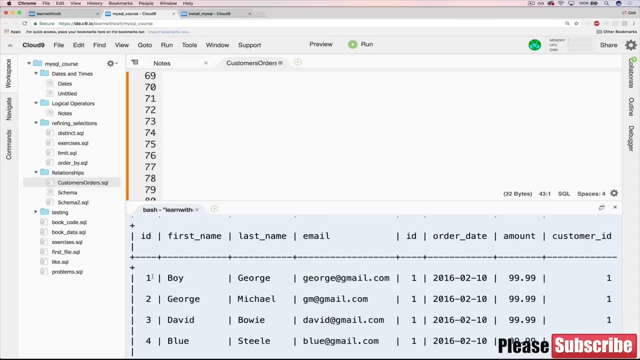 back to this really ugly cross join, where it takes everything and joins it together. So if I wanted to- there's no meaning to be garnered from this- but I could join it where the two ids are the same, So not customer id, but I could say where customersid is the same as. 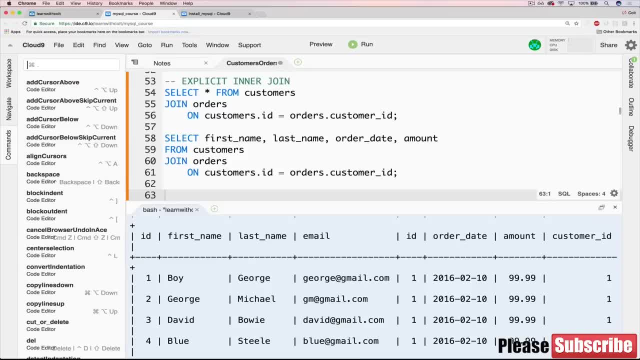 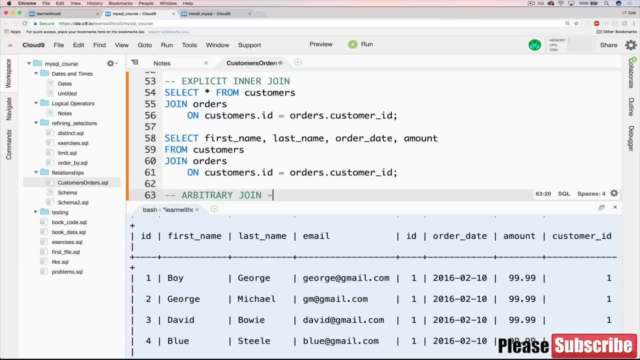 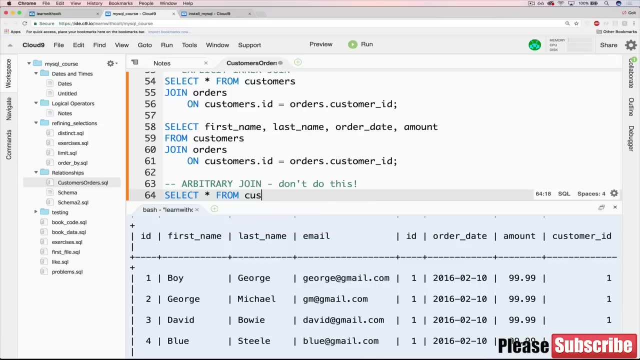 ordersid. So let me just show you that now And I'll just comment this as arbitrary join Don't do this. But we could do this. We could select star from customers join orders on and I'll just say where customersid equals. 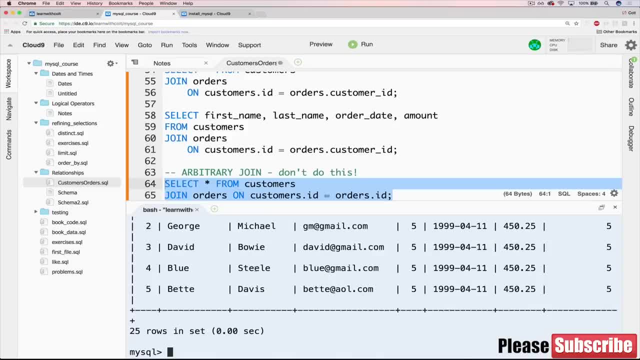 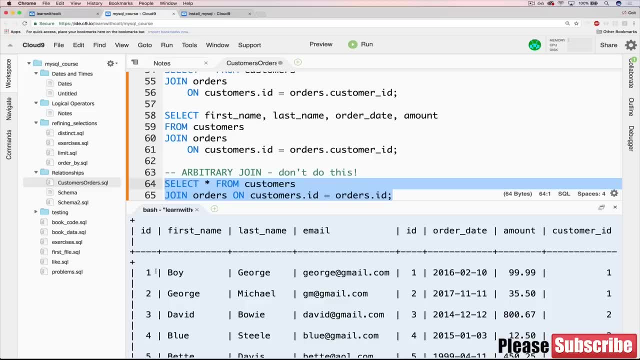 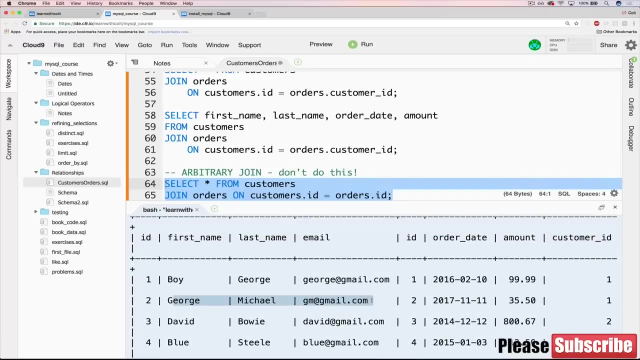 ordersid. There's nothing stopping me from doing this And, as you can see, I just end up with this new table that has matching ids. So we get- let's take an example- like George Michael. So George Michael is now matched. He has an id of 2.. He's matched with. 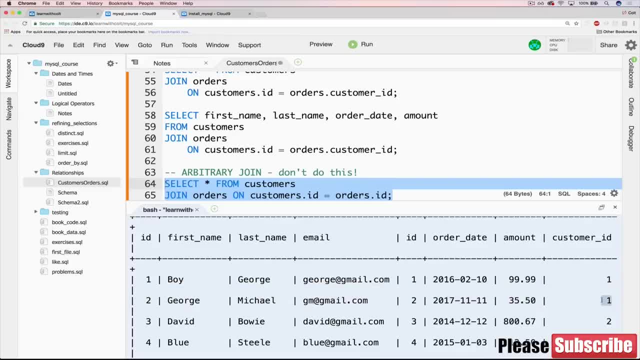 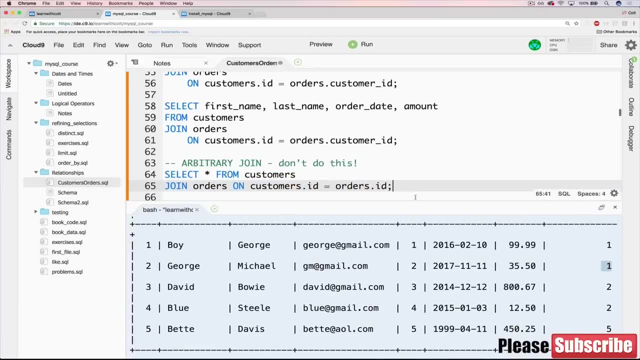 the order of id 2.. It doesn't matter that it was placed by customer with id of 1, which is boy George. So I'm saying that we can just join things on arbitrary conditions. However you typically what goes in here is you're filling in a foreign key. 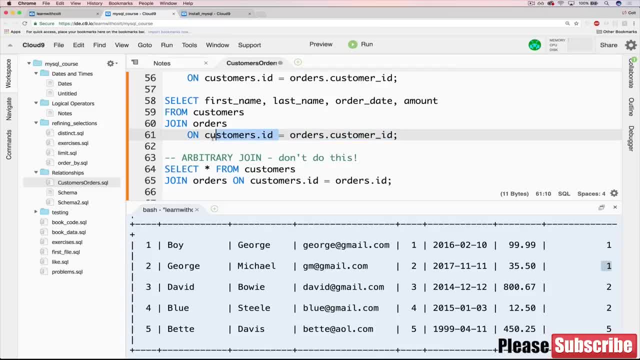 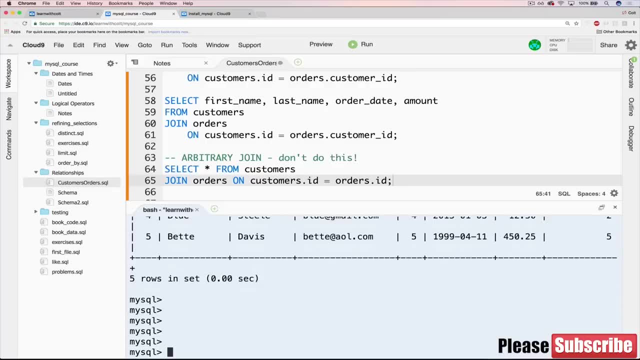 matching a primary key in another table. So primary key is the customer's id, The foreign key is the customer underscore id in the orders table. And then the last thing that I'll wrap up with here is: does the order matter? So if we go, 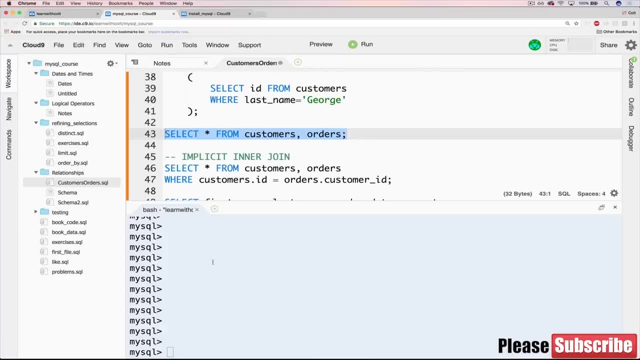 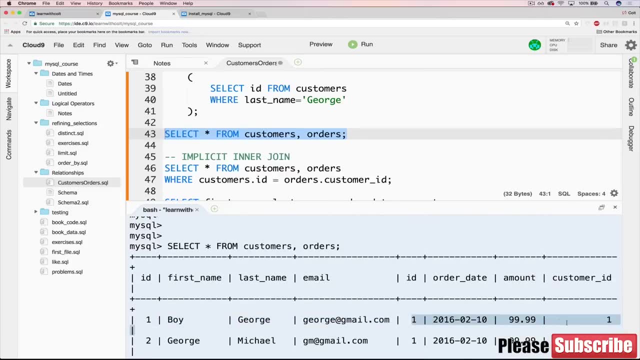 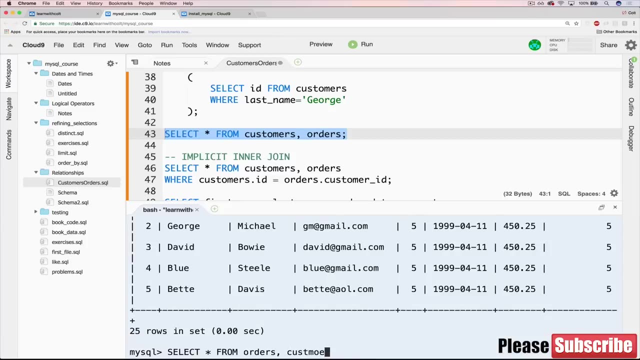 back to our cross join. what if I reverse the order? So I started with customers, comma orders And so we get customers here and then orders tacked on on the right. So what if I switch it- Orders, comma customers And you can see, well, it looks very similar, except, well, it doesn't look similar. 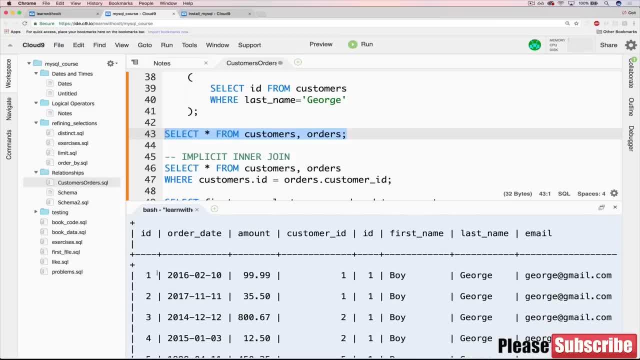 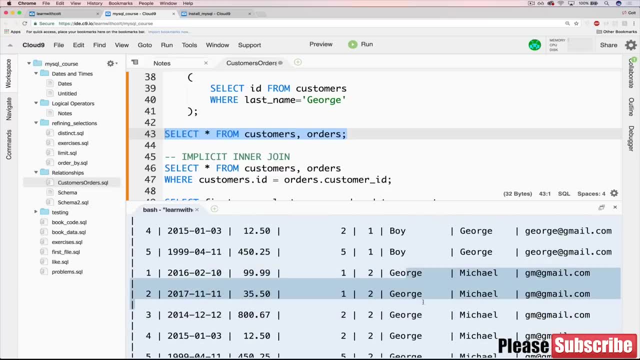 We have the same data but it's been switched. So we start with every order first, and then one customer tacked on to the end, And then every order again and then the same customer. So the order does matter, in a sense, as to how your data is presented to you. 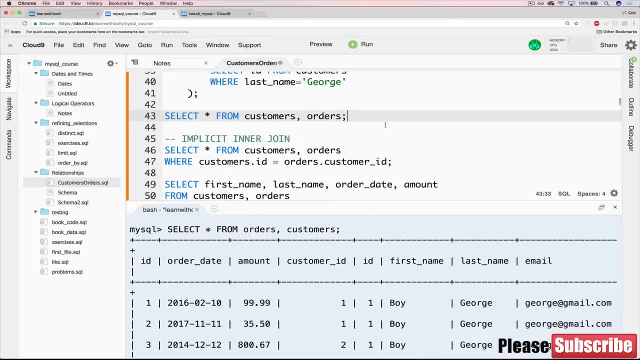 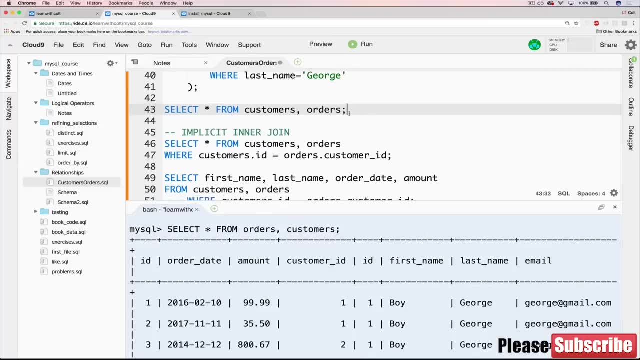 But it doesn't matter. in the case of a cross join or in the case of an inner join, It won't actually affect the result, It just affects what is printed out, what it looks like. So let me show you. If we take this same, we've got a lot of them. 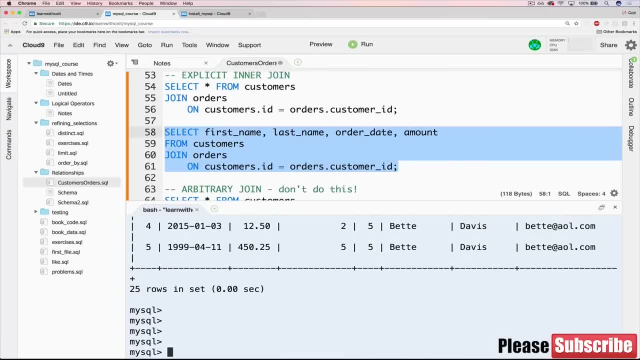 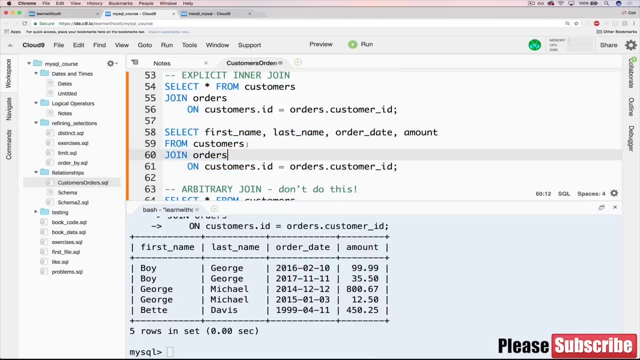 going on here. Let's take this same one here. This is kind of the most useful join we had right, Where we had the name and the order date and the amount. If I switch- and I'm just going to duplicate it so that we have the original as well- If I say from: 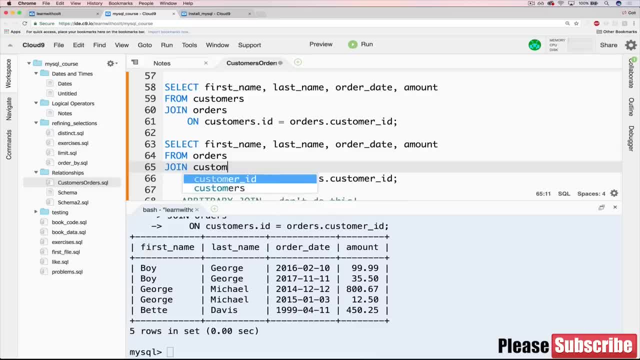 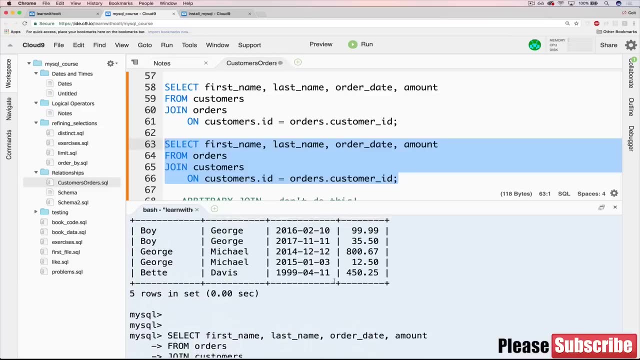 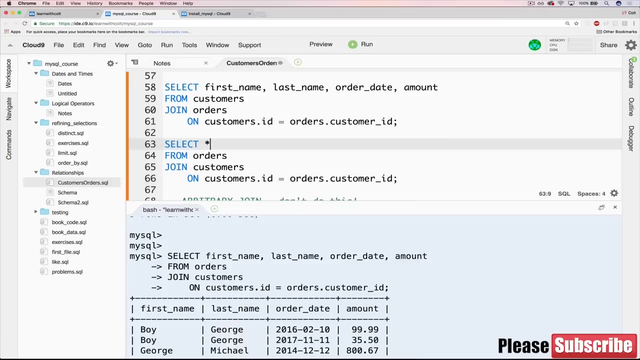 orders join customers on and we can leave this either way. But let's say I do that, So I'm selecting from orders with joining customers on to it And I hit enter. Nothing changes And that's because we are picking our data individually from up here. Now, if I just did a star, 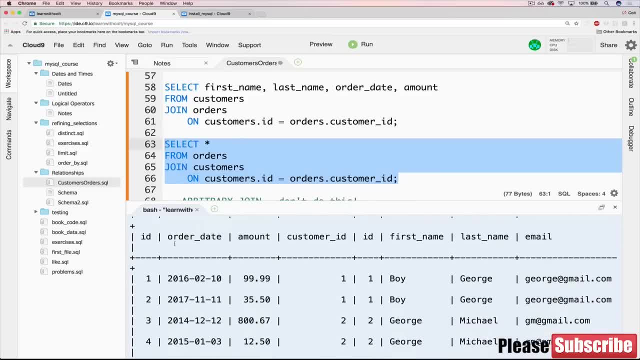 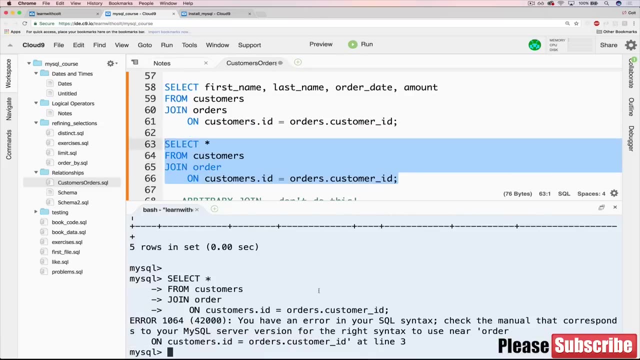 it would look a little different because you can see we're actually getting order first, So order ID, order date, amount and then customer. And if I switch that it would be the other way around. That doesn't really matter, It's just: oh orders. 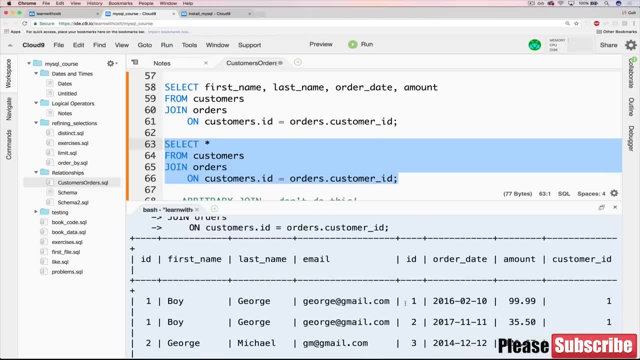 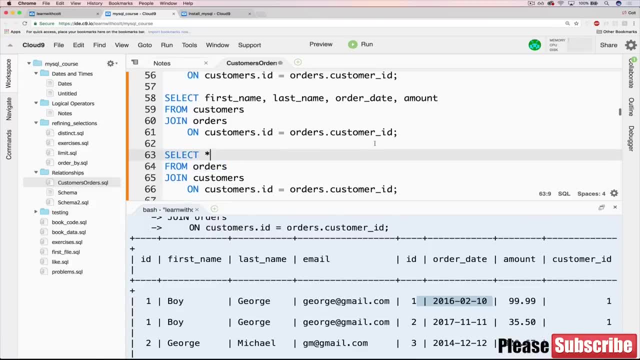 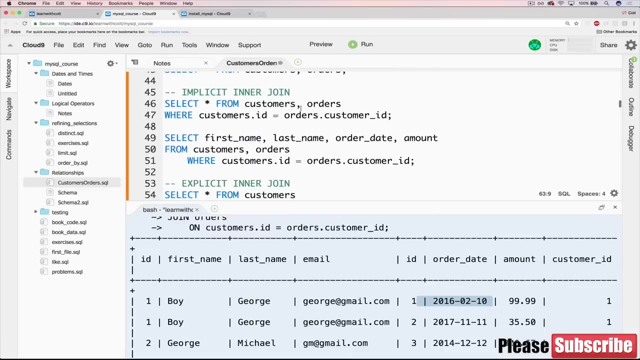 But you can see now we get customers and then orders, Alright. so this has been long And a little difficult, I imagine, Especially some of the syntax or keeping the jargon. What I do want to say is that, basically, when you're joining, things don't do. 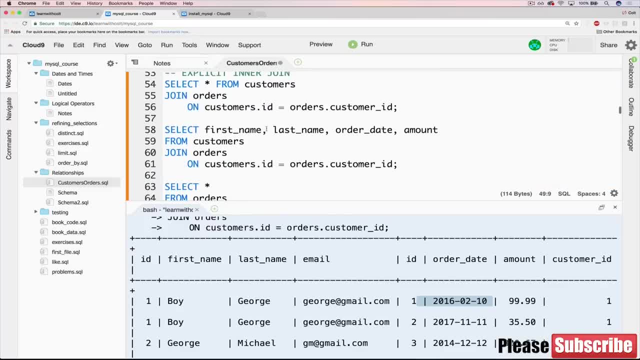 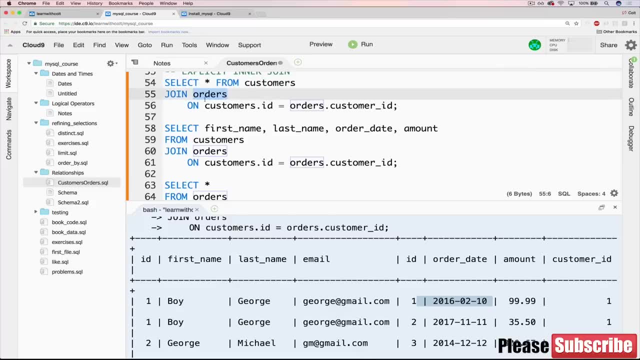 implicit joins, which is what we have here. It's better to do it explicitly this way, So something like this or this, where we have select something from a table, join on another table on a condition. Okay, so that is kind of. 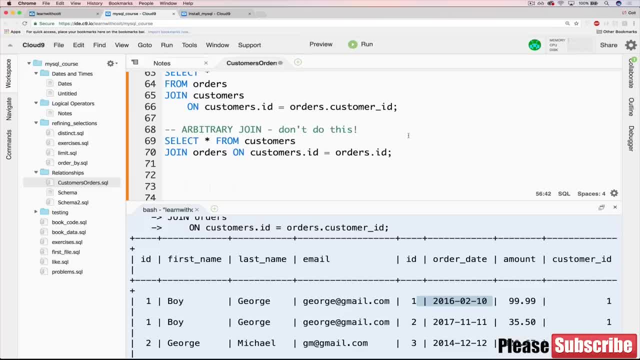 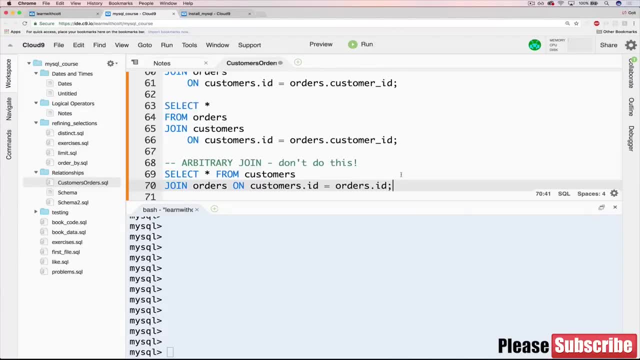 the bread and butter of joins doing an inner join. But I'm going to show you a couple of other examples That will be up next. Okay, I hope you're still with us. I really hope I didn't put you to sleep with the last video. These are getting. 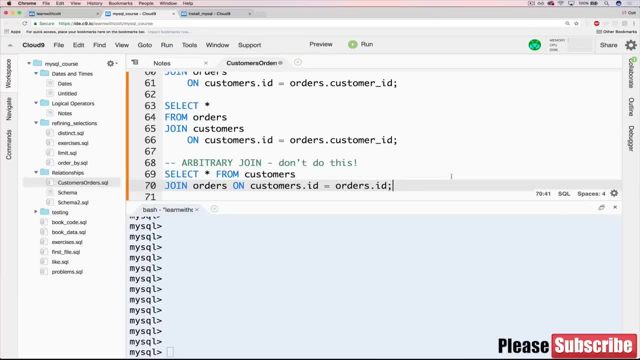 a little too long for my taste- Significantly too long- So I apologize for that, But there's a lot to cover here And there's no great place to break it up. However, we are done with kind of the long slog of explaining joins. Now I'm just going to show you another type. 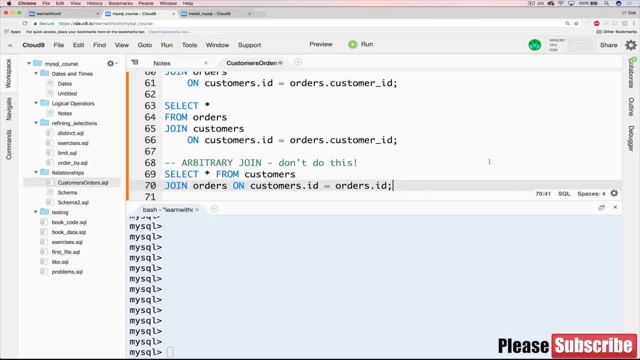 So inner join is what most people end up doing. That's a big generalization, But it's what I end up doing most of the time. But there are other types, And the next one that I'll show you is called the left join. 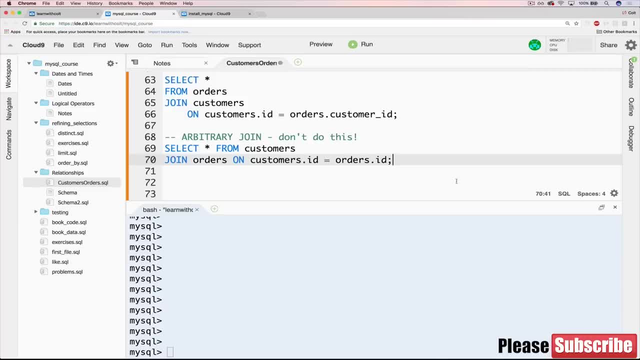 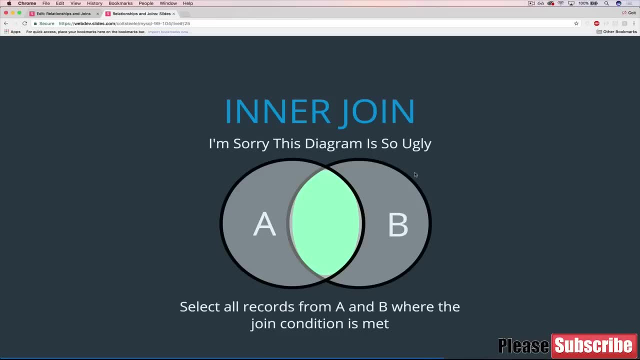 There's left and right, They work very similarly. So once you understand how one works, it makes it easier to understand the other. So what we saw so far was the inner join, where we take one table A and another table B, And then we 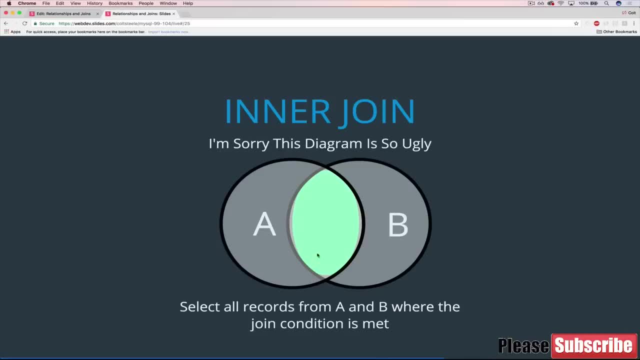 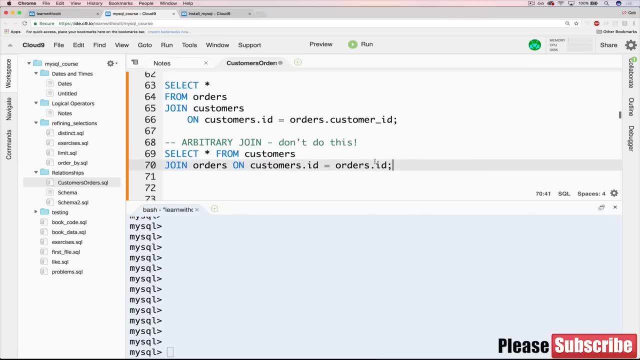 select all the records from A and B where the join condition is met. But there's another type of join. Before I get there, I want to show one other thing. If we go back to any of our joins that we had, let's take this one here. 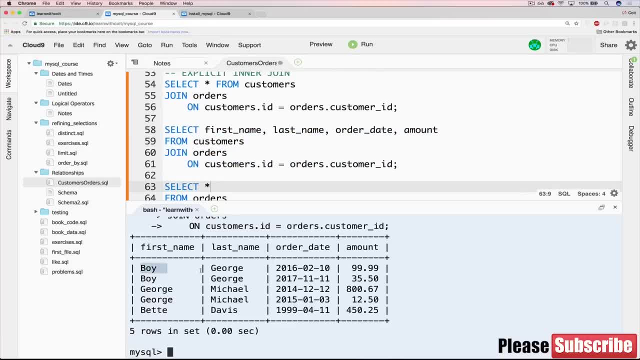 So this gives us our nice little table with boy George and his orders. We have George Michael and his orders and Betty Davis and her orders. I can do just any regular MySQL functions and things that you're used to with this data. So I didn't make that very clear in the last video. This isn't some special table. 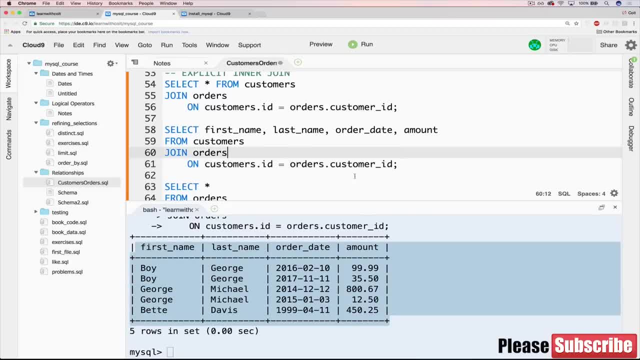 We can do whatever we want. So I could do something like group by. Or- let's start even simpler. I could do an order by. Let's do an order by. Let me actually move this. so we have a record of everything we've done. So 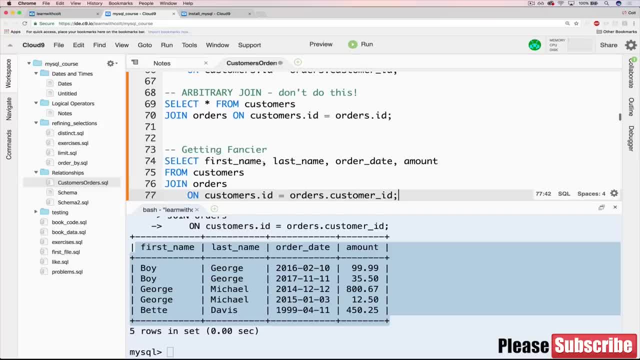 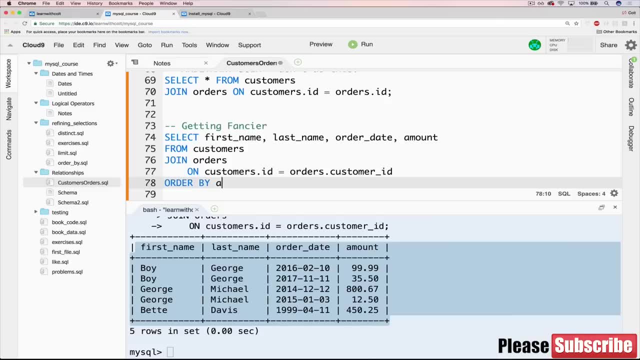 I'll scroll down, Getting fancier. Here we go. So we can do an order by amount if we wanted to, And now we have from the lowest order up to the highest order, Or we could order by order date. So that's one thing we can do, But we can also do things. 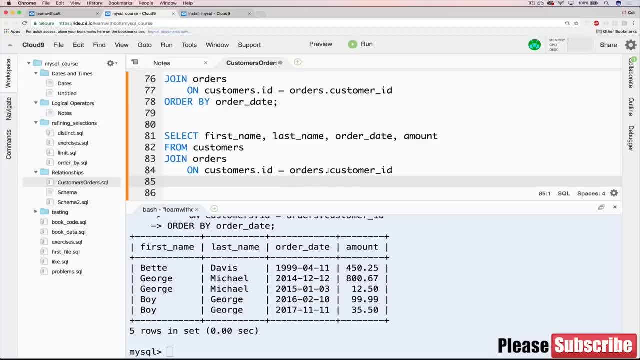 like group by. So maybe let's say this is something we actually might want to do: is take all of our orders and group them by who ordered them. Okay, Group them by who ordered them and then take that and find the average amount they spent Or the total amount. How about we start? 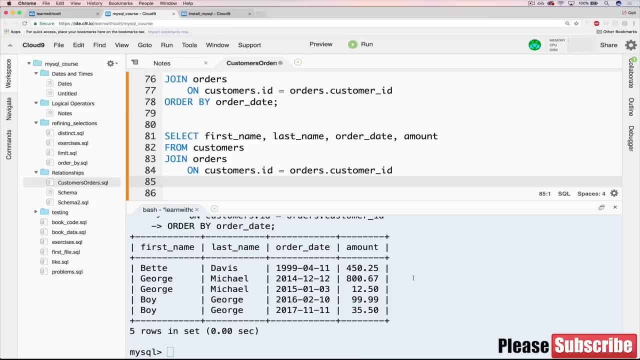 there, Let's identify the biggest spender in our entire database, Which is pretty easy to do if you just look here and add things up. But let's say we had 10,000 records, How do we find the biggest spender? So we'll group by: 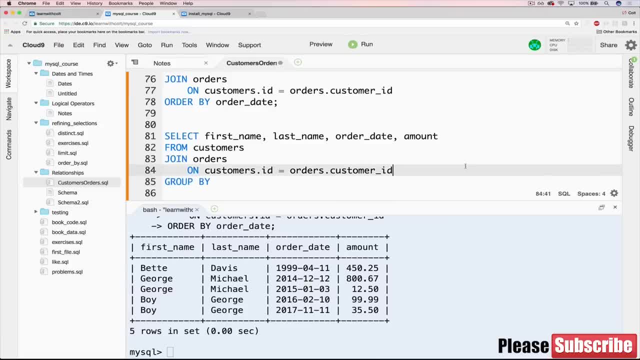 And how do we group them? Well, we want to group by our customer Place. the order First name could work, But that assumes that we only have one Betty or one George, And we might have George Michael and George Foreman or something. So that's. 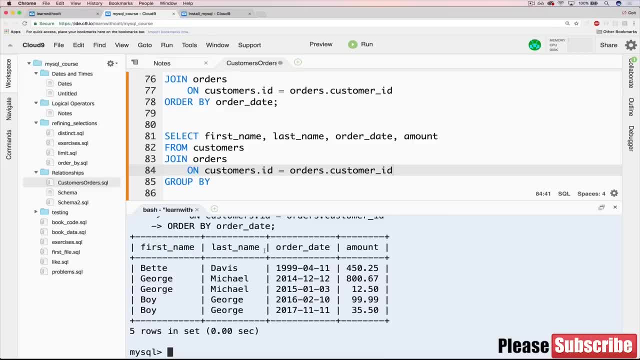 not going to work. We could do first name comma, last name, But we still could have people with the same name. So it's better to just group by something we know is unique, Like customer ID, Just like that, And let's be explicit: Orders dot- customer ID. 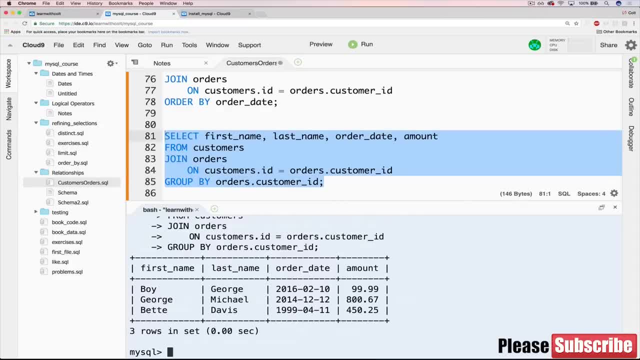 So group by that And if we hit enter, remember when we do group by and we don't actually do any math or any functions on it. It looks like it just cut data out, Because that's just how it prints things to us. But now you can see that we have grouped. 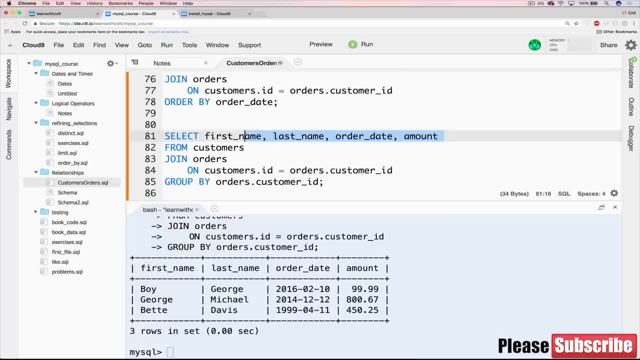 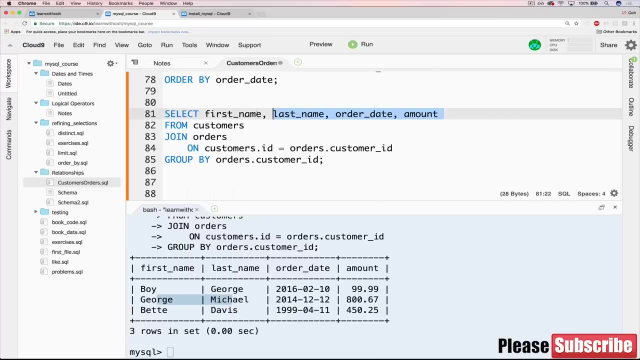 by the customer ID. So I know it's hard to see because we're not displaying customer ID, But remember that customer ID is unique relative to every user. So we're basically grouping by customer. Hopefully that makes sense. You could make it a better. 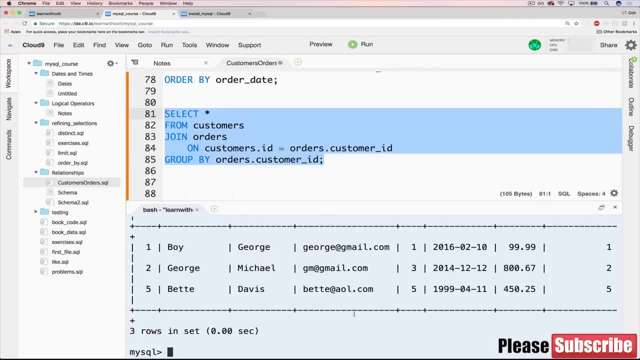 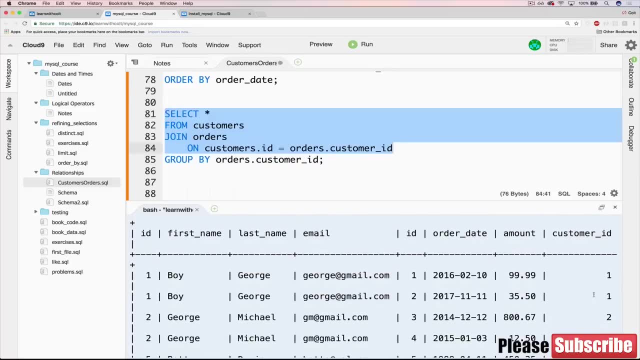 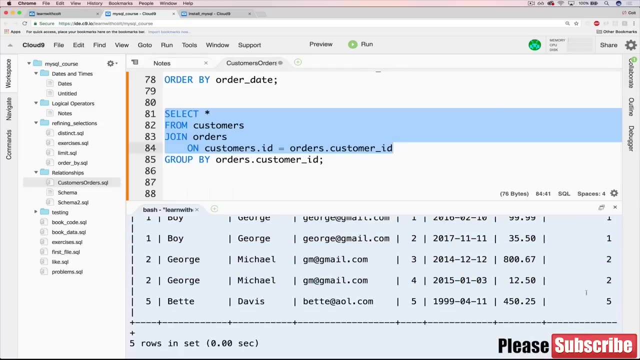 bit clearer if you did something like this. What we've done- And let me get rid of the group by Briefly, What we've done- is take these customer IDs here that we weren't showing And just grouping these two together. These two together And this one on its own. 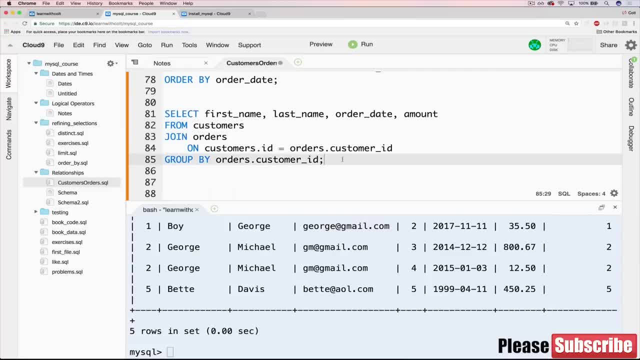 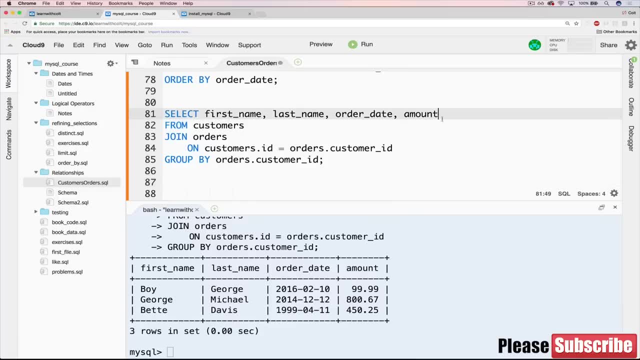 But we're not actually displaying that. Okay, So we can group by that, Like we did, And then all we want to do is total together the amounts. So, rather than just amount, let's do sum amount, And I'm going to clean this up a little bit. 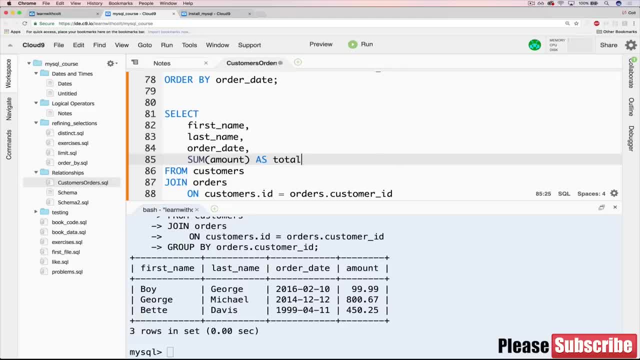 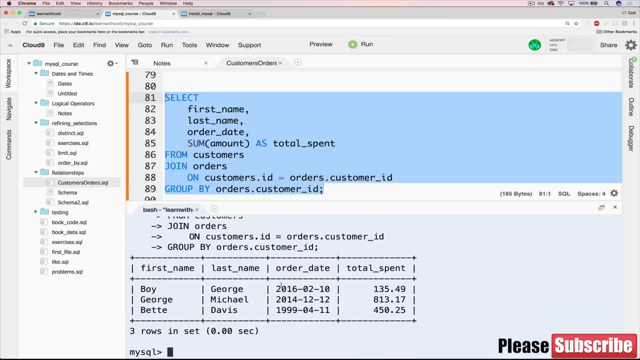 And let's give it an alias as total spent, Just like that. Now, let's try it. Cool, So we can see: Boy George spent 135.. George Michael 813. And Betty Davis 450.. And then, lastly, we could order by total spent. 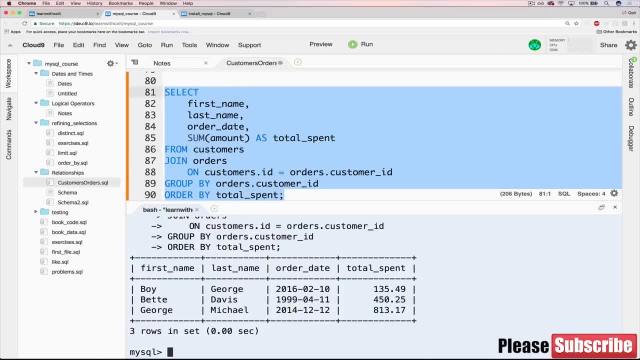 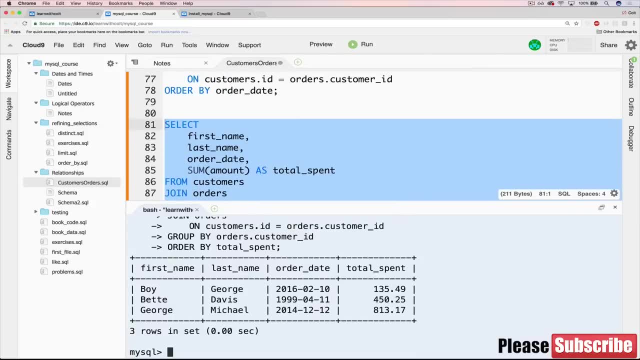 Move our semicolon. Now you can see. And actually let's do descending. Now you can see. Okay, George Michael is definitely our biggest spender: 813.17 cents, Perfect. Now, the order date doesn't really make sense to have in there. So because we have multiple orders, 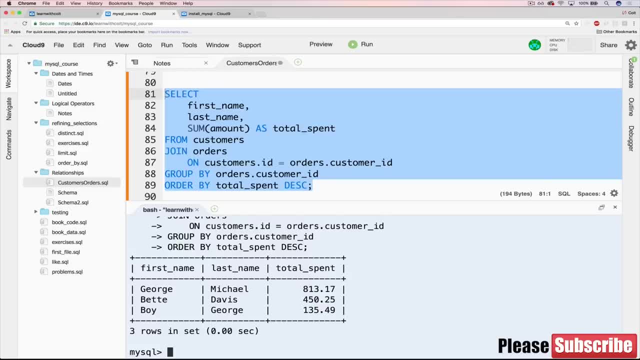 And it doesn't make sense just to show one, So maybe this makes more sense. There we go. Okay, So I just wanted to show that you can still do typical things that we're used to with the results of a join query. It's not some special alien type of a table. 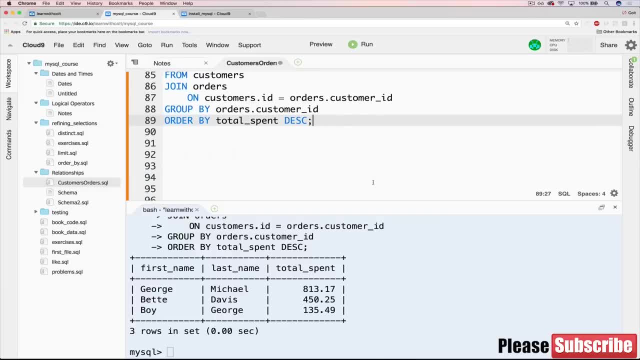 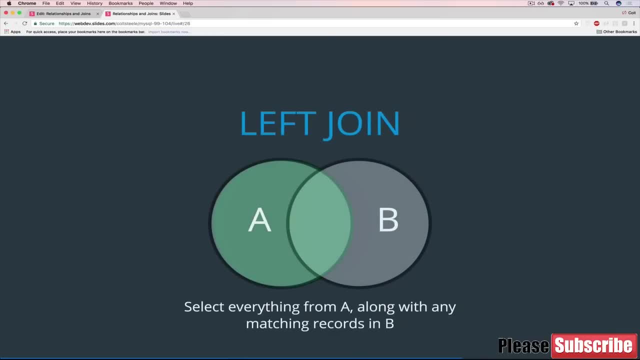 Now that brings us on to the left: join. So another way of joining our data. Here's the ugly diagram I tried to make. It's a little better. The colors are still awful, I'm sorry. So what does it do? Well, it's going to take everything from the first table. 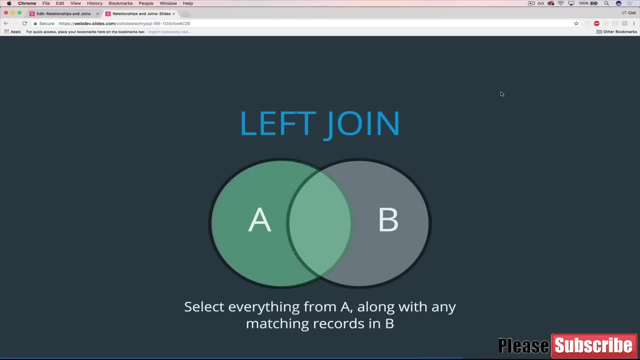 So if customers is our table on the left, It will take every customer And then on the right it will try and match, or it will match any or it will add any matching records from orders in our case. So these diagrams just talking about it like this: 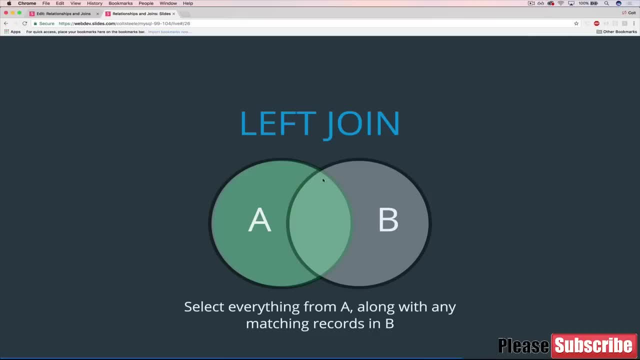 I find isn't that helpful. But basically think of it as it takes the union of where they match, just like inner, But then it also does everything from the left table, from customers in our case. So let's test it out over in Cloud9.. I have a comment here. 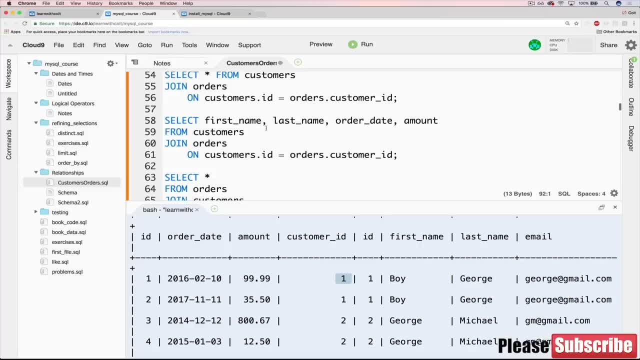 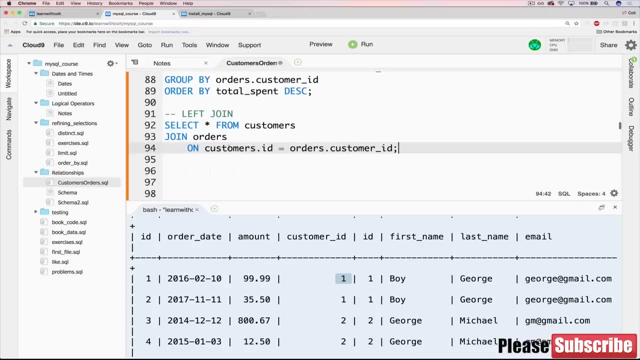 for left join And let's go take one of our joins that we did earlier, Like let's do this first one. This was an inner join, And one thing I didn't mention is you can explicitly write inner join And I'll show you. 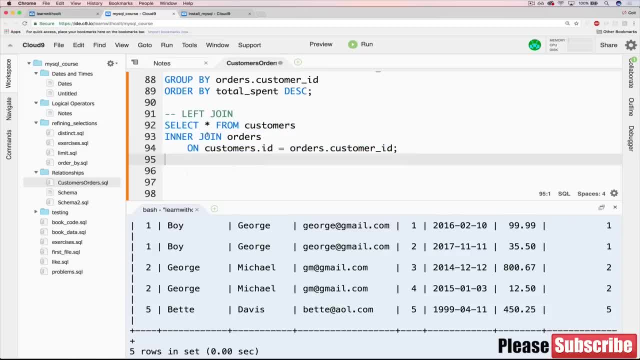 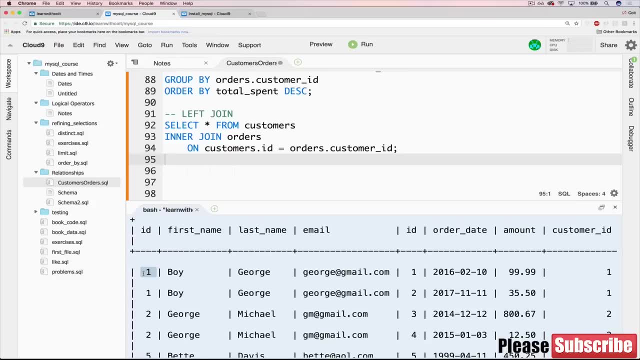 It does the exact same thing. If you leave it off, it's implied that it's going to be an inner join. It's the most common type. What it does is: we know it takes customers where their ID matches customer ID and that's all we get. That's the inner part that matches. 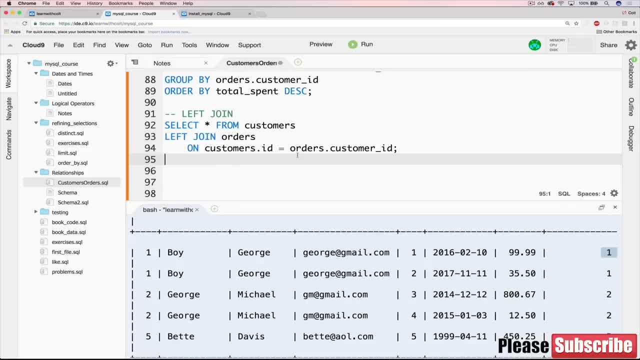 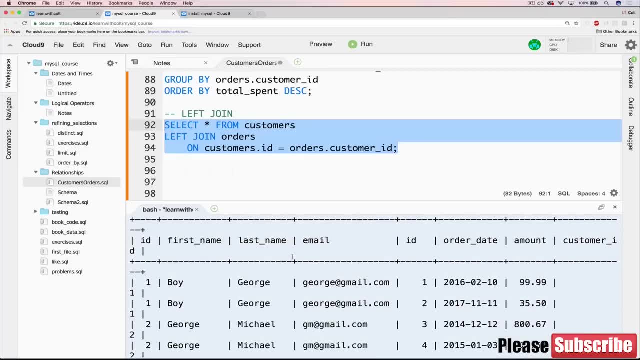 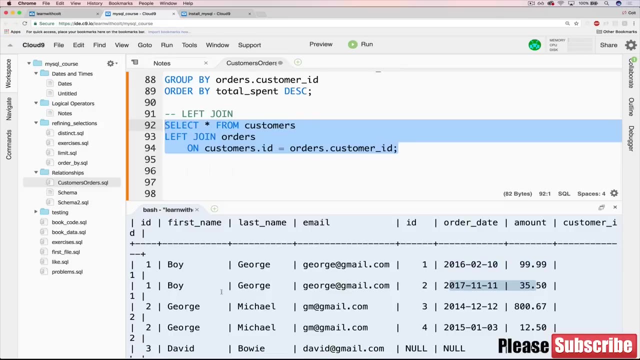 Now if we change this to be left and select everything, You'll see we get a couple of differences. So we still have. Now it's kind of ugly to look at. I'm sorry. We have boy George in the order he placed and boy George- another order he placed. George Michael, two orders. 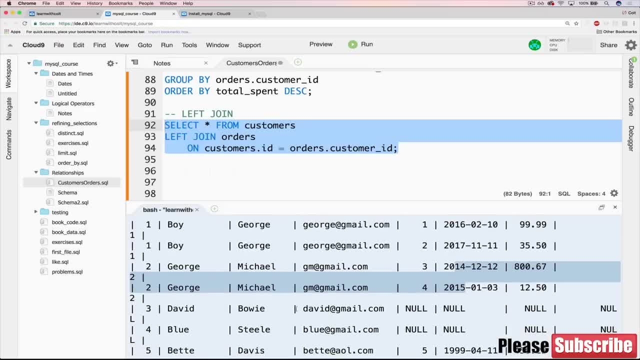 that match. But then we have two users who never placed orders. David Bowie and Blue Steel do not have orders, And so we end up with David Bowie, Blue Steel: null, null, null, null for the orders portion, And then Betty Davis and the order that she placed. 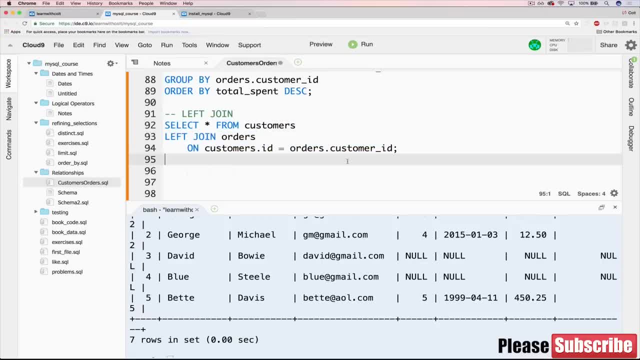 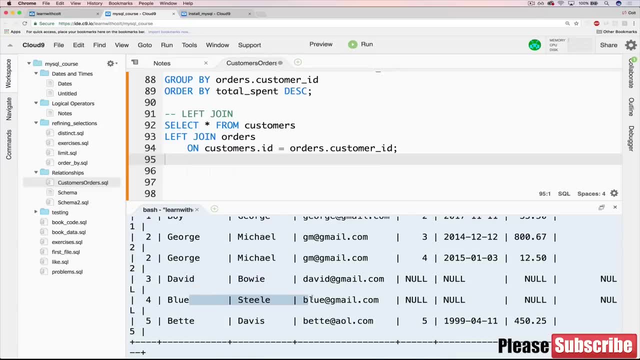 So we have customers on the left, Orders on the right. We're taking everything from customers. So that's why we end up with David Bowie and Blue Steel, And then we take the intersection as well, where there is an applicable match. So for David Bowie and Blue Steel there isn't one And it fills in null. 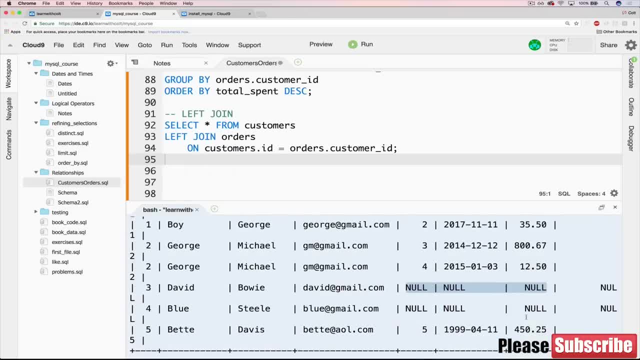 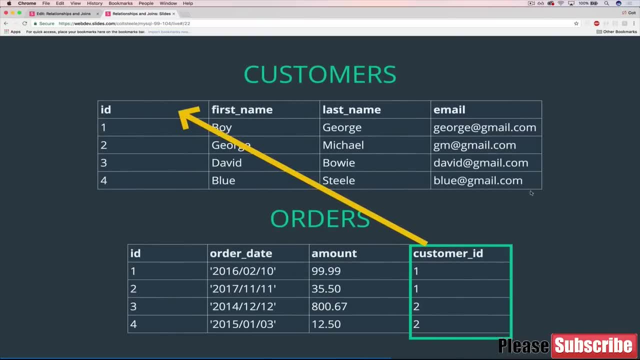 But for boy George and George Michael and Betty Davis there is a matching order. So I know it's kind of difficult to look at or understand. But think of it again: We have customers And we go through at the beginning. Okay, Boy George. 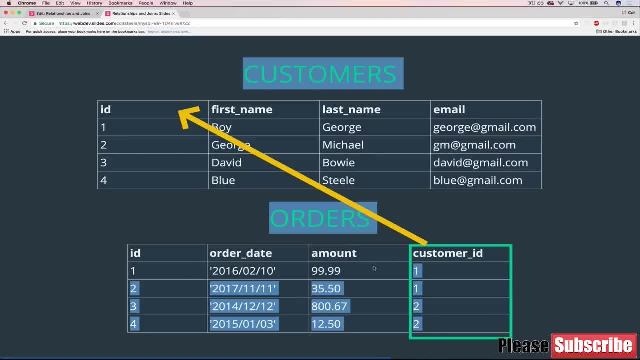 is there a matching order? Yes, This one here, Right here, And this one, So put those together. George Michael- ID of two. Is there any matching orders? Yes, There's two. Put those two together next to George Michael. 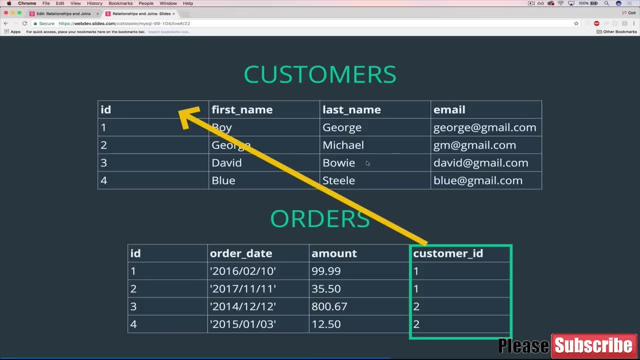 David Bowie. Is there a matching order? No, So just put David Bowie, because it's a left join. If it was an inner join, then David Bowie and Blue Steel don't show up, But it's a left join, which means we're taking everything from the left table And it works perfectly. 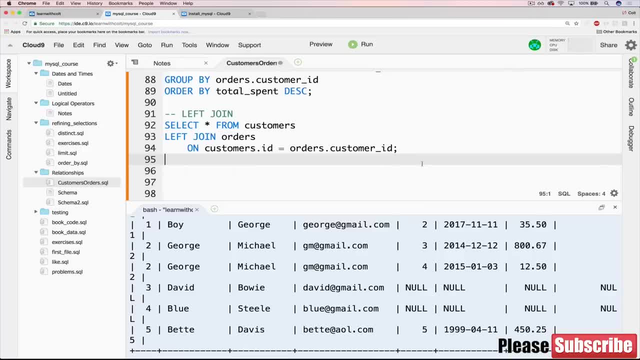 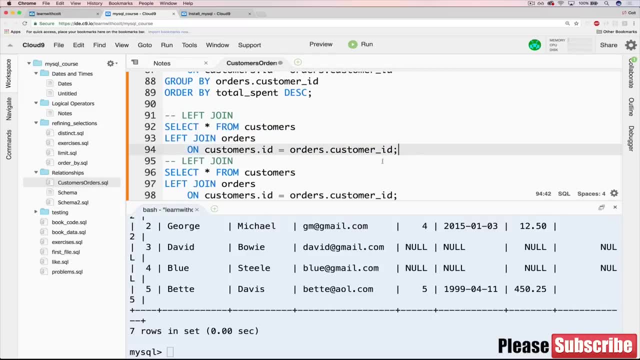 Well, depending on what you're trying to do. So that brings us to the question: why would you do this? And before we get there, I'm going to just clean this one up again so that we can see it a little bit easier. Let's only select first name. 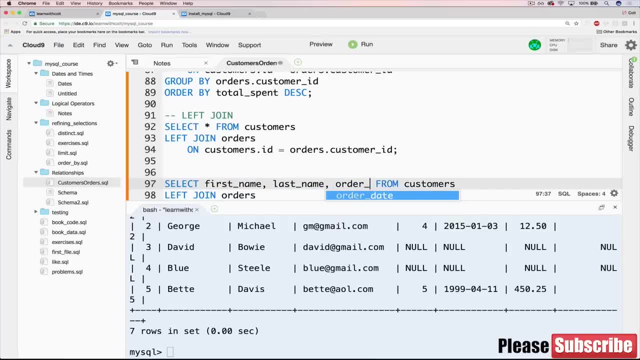 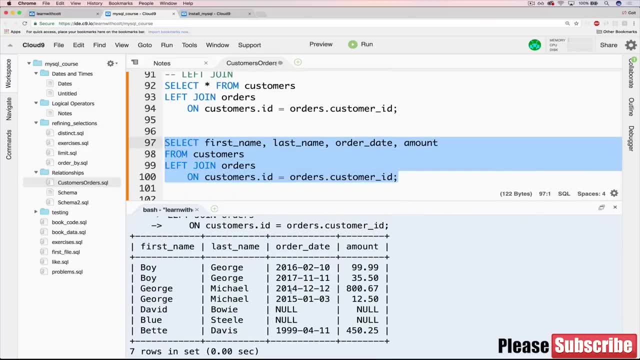 last name, order, date and amount, just like before. So that brings us again to the question: why would you do this? Why would you want to have excess information, like David Bowie and Blue Steel? And it depends on what you're doing, And in this case, maybe I. 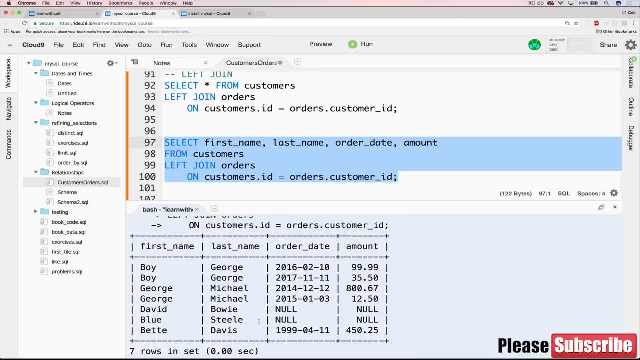 previously I wanted to see, okay, all the orders that have been placed and names next to them. But now what if I want to tabulate the high spenders on our site, but I want to include people who haven't spent anything. So I just want to be able to see for every user: how much have they spent? 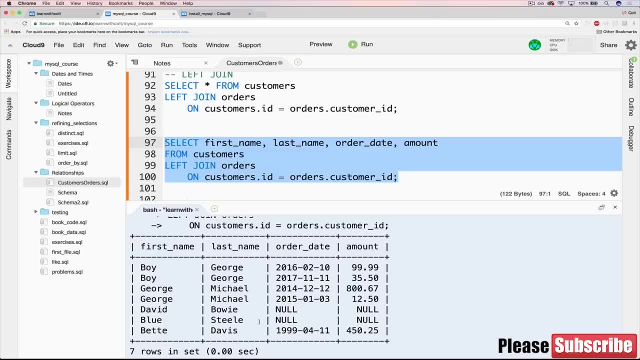 And I'd be able to go through and say, maybe send an email to the people who have spent a lot. Okay, thanks for being a loyal customer Versus people who haven't spent. I could go through and send an email like: here's a coupon for your. 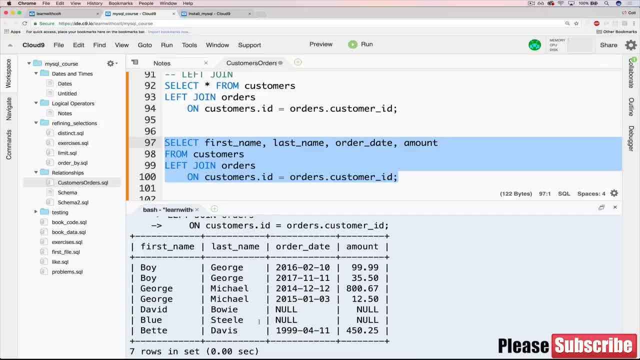 first purchase 10% off, Something like that. right, Where I want to basically get some insight, where it involves knowing everything about all users And some of them have corresponding orders and some of them don't. us to another topic, which is okay, but we have nulls here, so is there a way to change that? 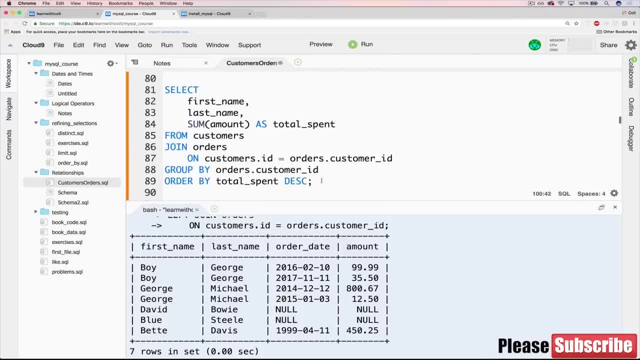 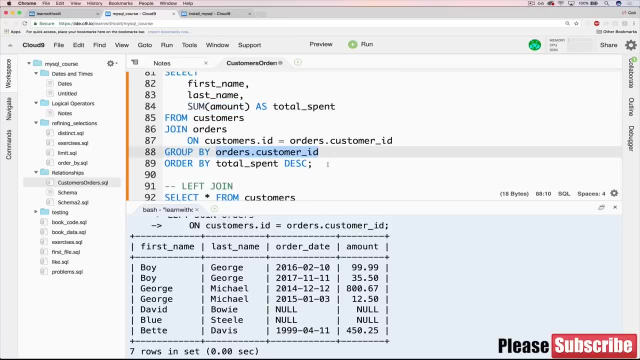 let's say, i wanted to do the same thing that we had up here, where we had our high spenders right, so we selected and we summed all the orders based off of grouping them by customer id. so it's a lot again, but let's do that here with a left join and there's going to be a slight difference, right? 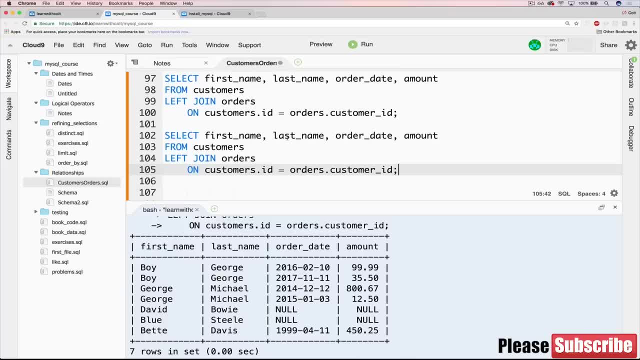 because we have nulls. so if we do this, select first name, last name, order date and amount from customers left join orders and we do a group by customersid this time, so that will group by customers, so that we have these two grouped, these two grouped on his own, on his own on. 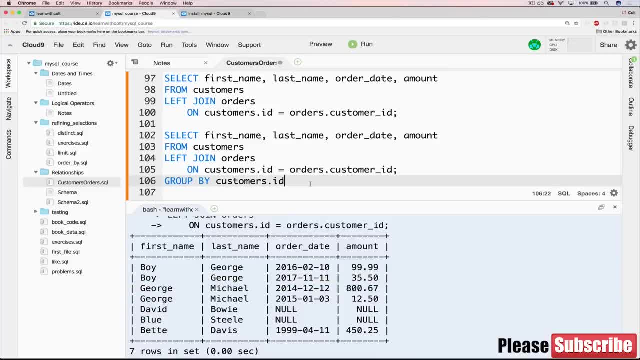 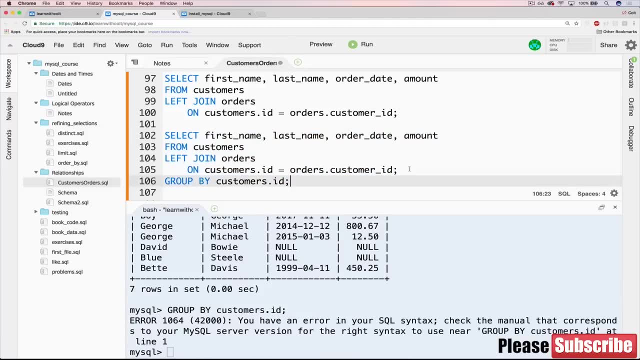 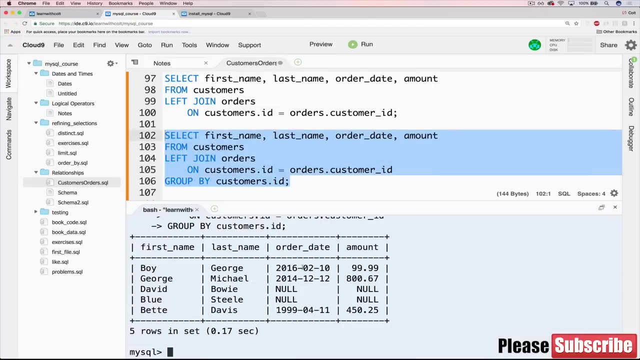 her own and actually blue is a girl, i'm sorry, blue. okay, so if we do this, we won't see much difference. well, we will see a difference, but it's not very meaningful. what am i missing? extra semicolon: not that useful because it just condenses our data and hides stuff. 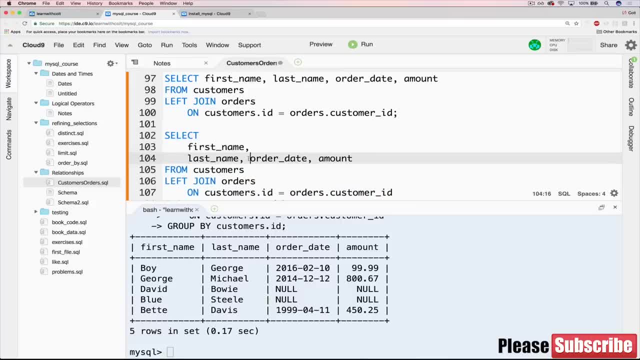 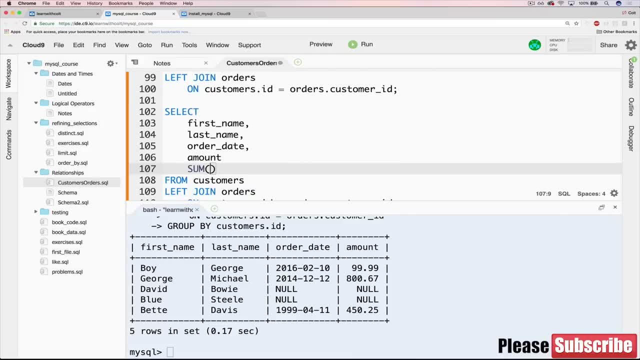 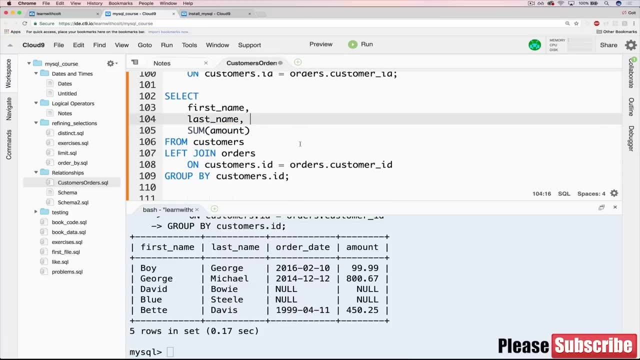 but if we go through- and i'll format this again- let's sum together everything, right? so we'll sum and inside of here we want to sum amount and we don't actually need to have amount there, and we can get rid of order date too. so let's just have the first last name and then sum. 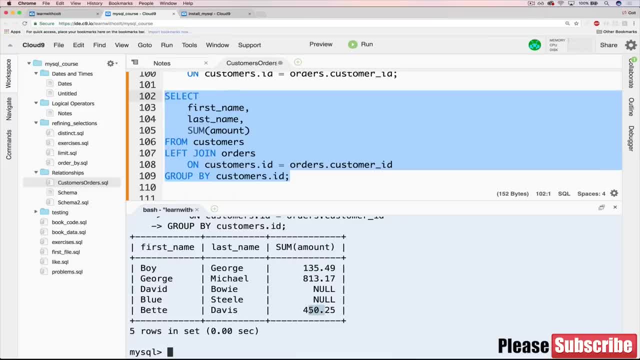 okay, so this is accurate. that's accurate. that's accurate. we still have null here, which it can work, but it would be nice if instead, it just said zero, because they've spent zero dollars. so how do we do that? and this is not an inner, this is not a joined specific thing in any way. 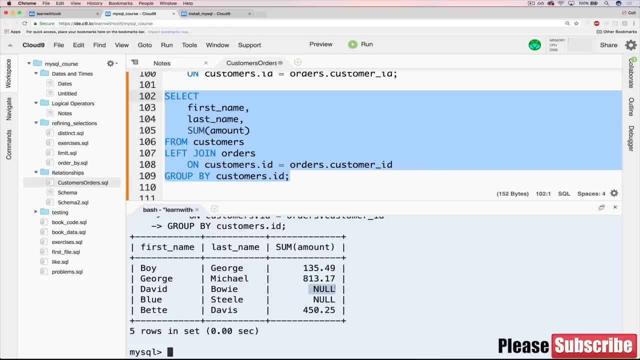 this is just an interesting problem: how do we get instead of null? how do i replace that with zero? and there's a couple ways. the first, really lengthy, awful way is to use a case statement. so i'm going. i could have a case statement where i checked: is sum amount is null, remember, i can't just say equals. 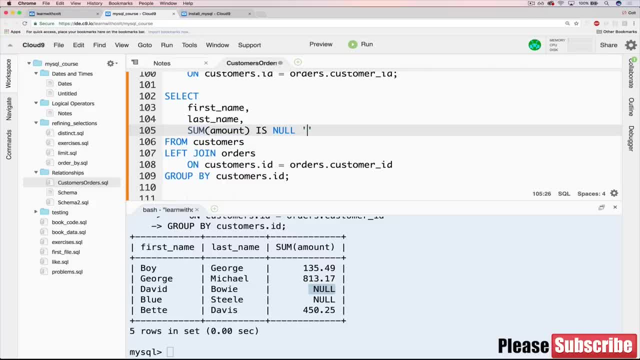 null. but if i said it is null, then do zero, otherwise do sum amount. but that's that's kind of long. so it's going to be much easier if i use what's known as if null, and i haven't shown this to you yet because we didn't really have many cases where we had null data. but here's one. so 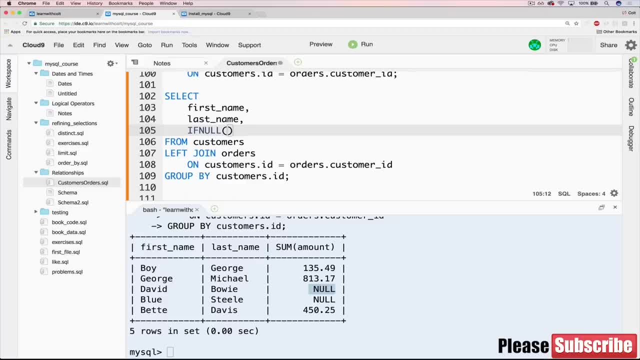 what if null does? it takes two arguments. if null does, it takes two arguments. what if null does? it takes two arguments. the first one is the thing you want it to check, if it is null or not. so we want to check is sum of amount null. so here it's not right, it's not no, it's not no. 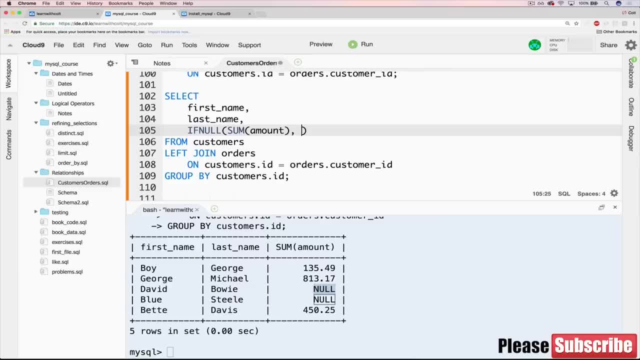 here it is. so then the second argument is what we want to replace it with if it is null, and we'll just say zero. so it's very simple: it checks if the first argument is null. if it is, it replaces it with the second argument. if it's not, it. 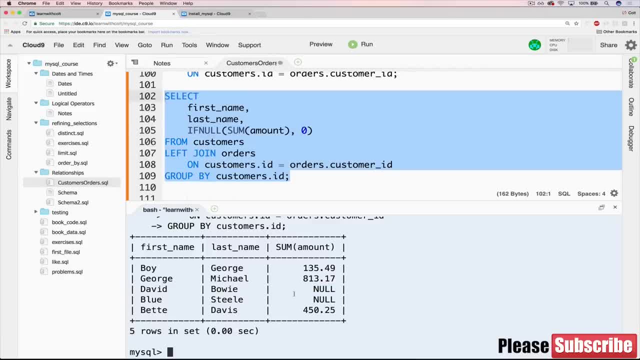 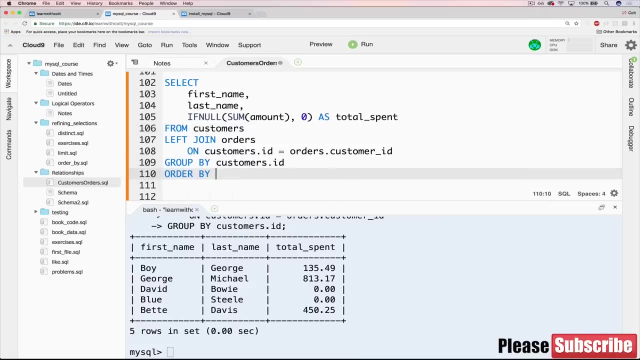 leaves it as the first. so now, if I try it perfect, we get zero. we should definitely add an alias. let's call it total spent again. okay, one other thing that would be nice is to order by total spent, and this time let's do it from least, so we'll just do order by total spent, and that should work. there we go. 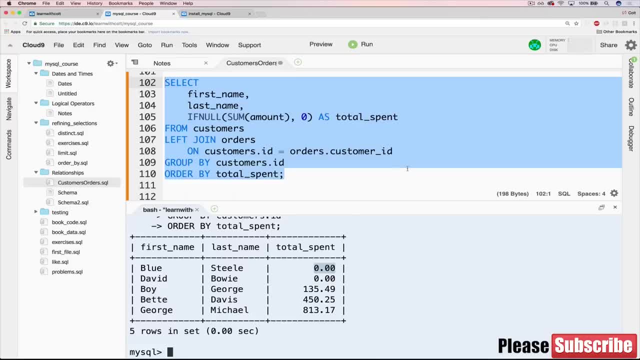 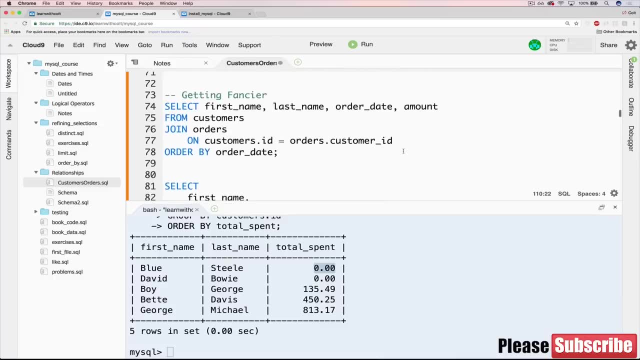 and now you can see we have zero. okay, so I we kind of talked about a lot. there's a couple topics that touch on each other. the first thing, just to recap, was that I wanted to show you when we do joints- any joints, they're not fancy special tables, they work just the same. 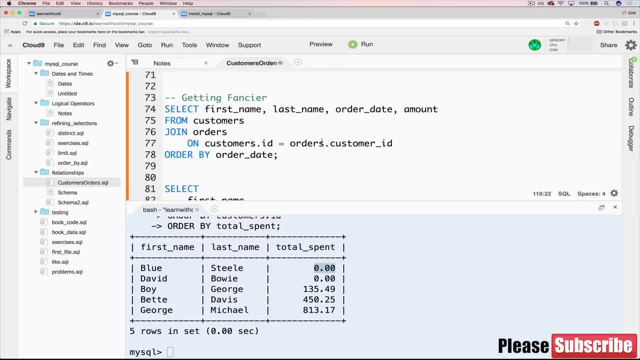 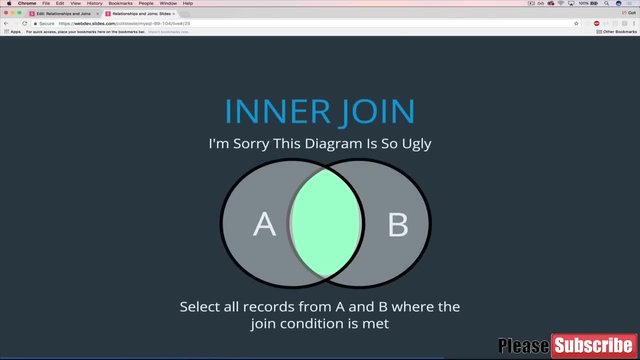 way as any other table, so we can do things like group by an order by then. the next thing was that we saw inner joints. if I go back, we saw this and we also saw a left joint and the key joint is the left joint and the key joint is the. 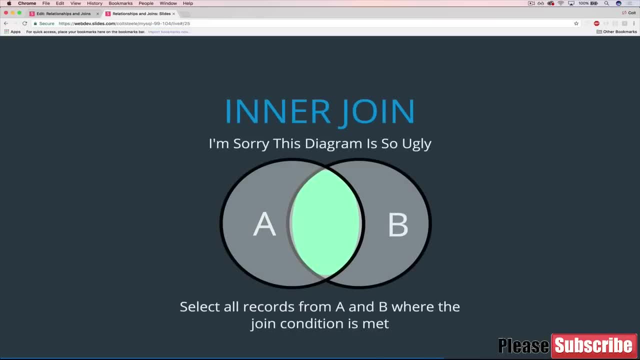 right joint and the key joint is the left joint, and the key joint is the left joint and the key joint is the left part of the left joint, and so that's the key difference. they both join data from two tables, but the key difference is what data they join. so we give them a condition. but even given the same, 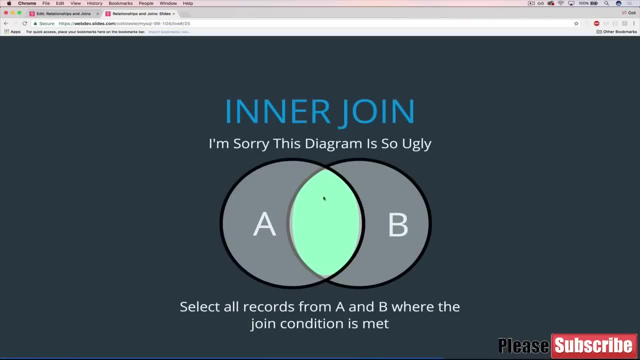 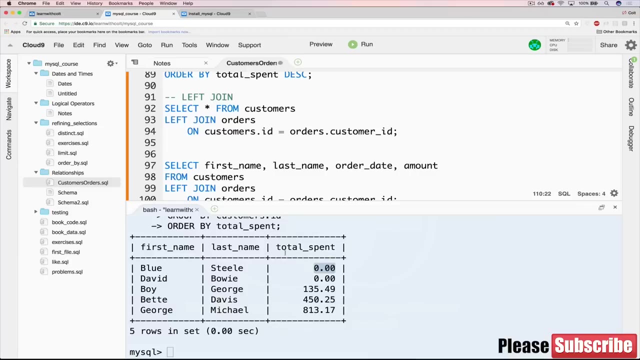 condition. in our case it was: join on customer ID equals orders dot, customer ID, this middle part and on inner join. that's all we get is the exact overlap. on a left join, we also get the left part in addition. so every customer in our case, which can be useful if we wanted to see things like which customers had an 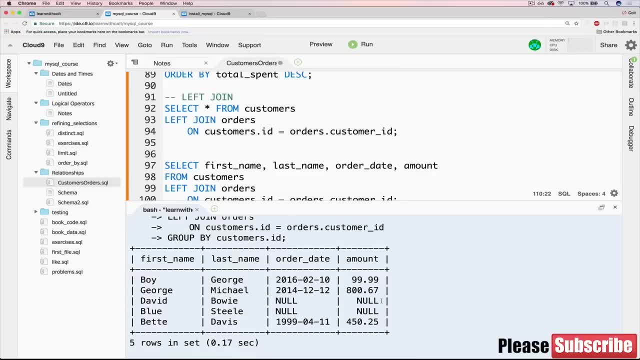 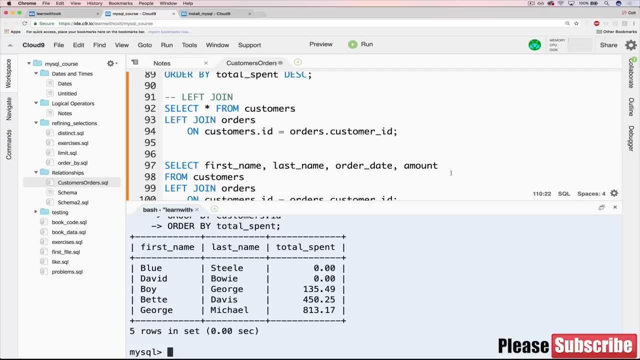 ordered things, which is what we got here. so hopefully that explanation made some sense. I totally understand if it didn't. it's. this is a tough, a tough thing to really wrap your head around at first. now it's not terribly difficult once you get going with it, but understanding it, it can be super intimidating. so I if 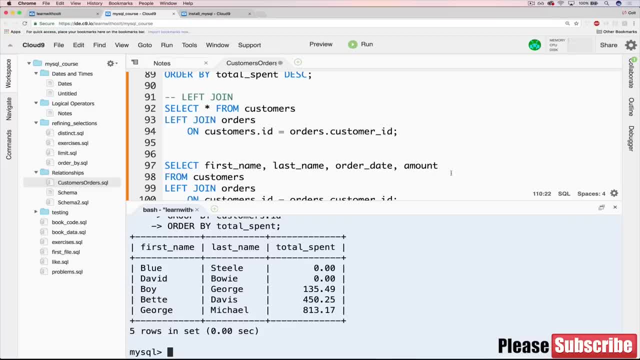 you're in that situation. we will have exercises coming up in just one more video after this and I recommend you try and go through those and if that's not enough, then absolutely ask for help in the forums here. this is one of the crucial things that, in my experience, sometimes 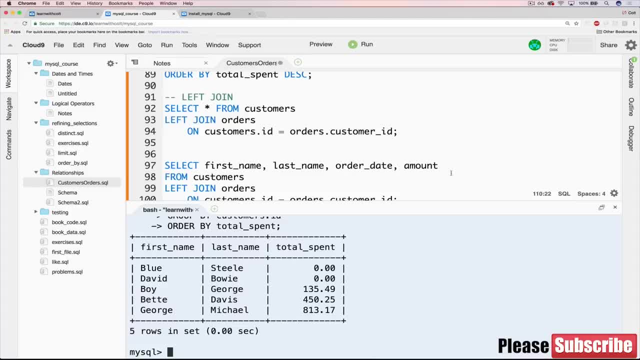 take students a couple of maybe hours, a couple of days, not not like 12, 20 hour days. I just mean sleeping on it once or twice to help kind of get some space in your brain. anyways, hopefully you're able to kind of get where I'm going with this. 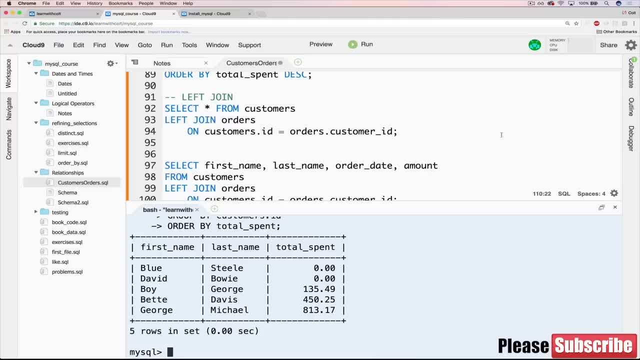 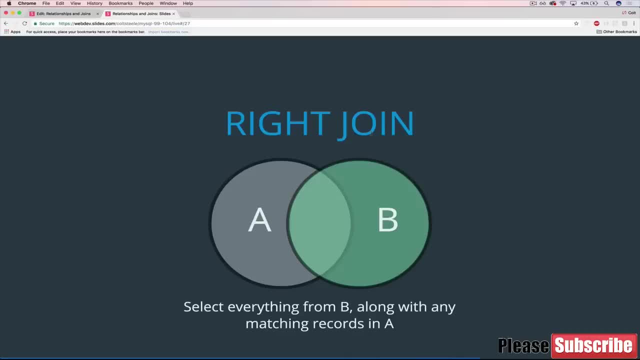 we're next up, we're gonna see our last type of join, which is a right join, very simple. come well, it's not simple, but very easy to grasp if you understand left joins okay. so we hopefully survived the last couple videos on joins. we had cross join, the. 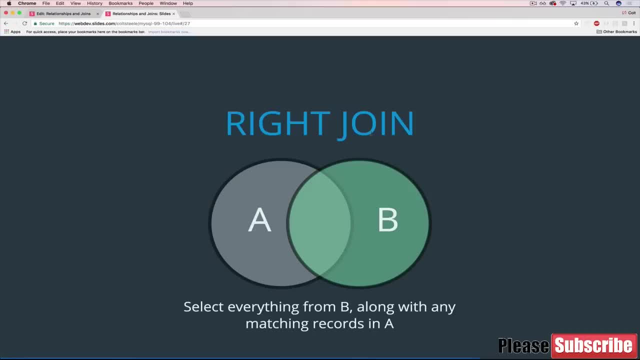 useless one. then we have inner join and then left join. now we have the sister or brother of left join, which is right to join. so it's actually this should be a pretty short video. it's very similar to left join in that it takes everything from one column along with- excuse me- it takes everything with from one table. 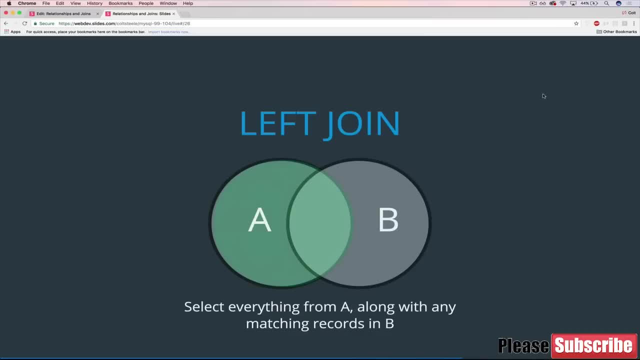 along with the intersection, along with where the join condition is met, but it just does it from the other table. so in this case we've been doing customers and then orders. so if we did a right join, it will take every record from orders along with any matching records from table a, which 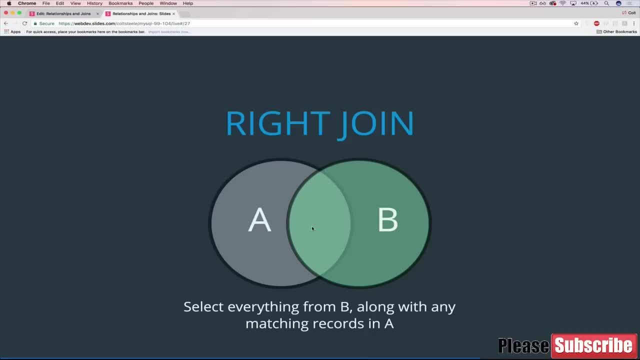 is our customers. now the thing is- you may have maybe thought about this already- we don't have any orders that don't have an existing customer, so we're actually not going to see it difference, But I'm going to come up with a way. I'll show you a way for us to see a difference. 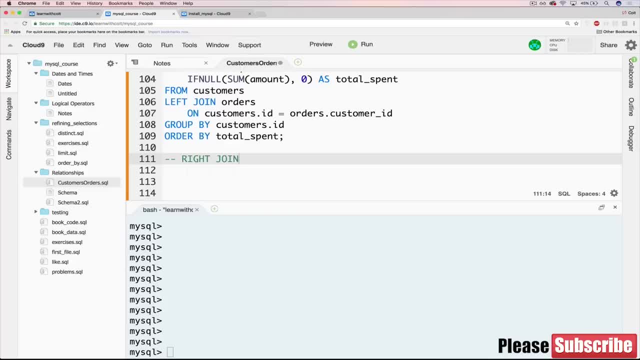 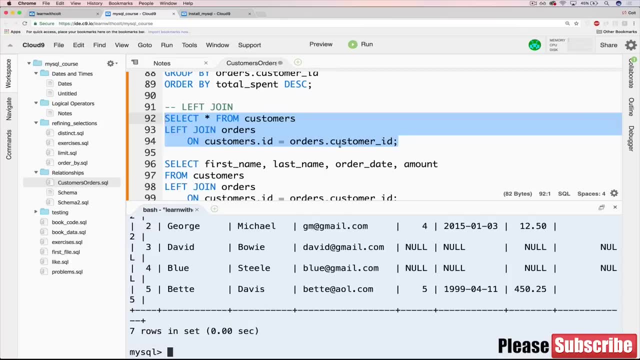 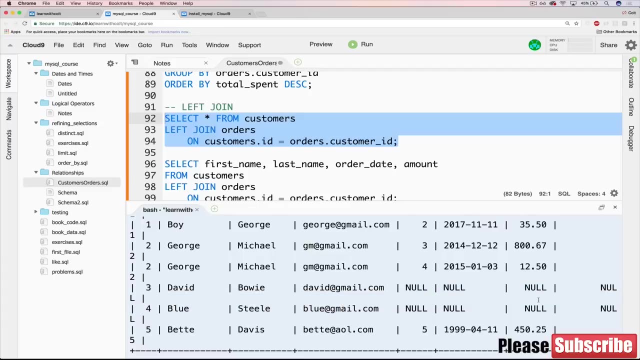 But to start, let me just show you the syntax. Okay, so let's hop over to Cloud9.. And here's our simplest left join that we wrote, Remember it does this here, where it includes everything from customers, David Bowie and Blue Steel included, even though they don't have any. 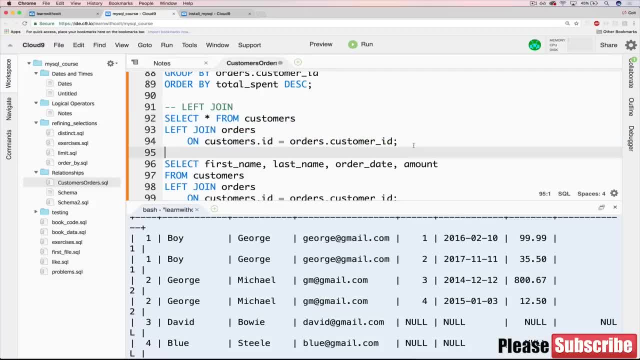 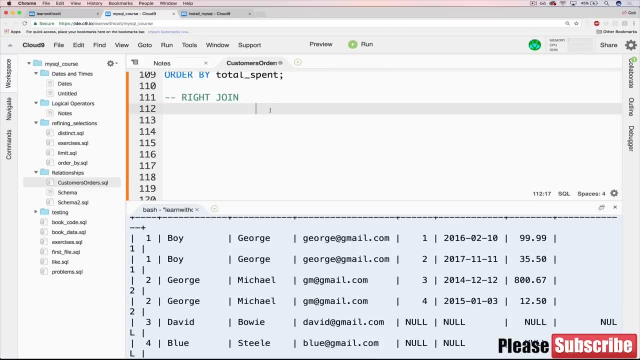 matching records And then it also includes all matching records. But rather than that, I'm now going to go and retype it down here as a right join. So we'll do a select, we'll just do star from customers And then we'll do join orders on customers. ID equals. 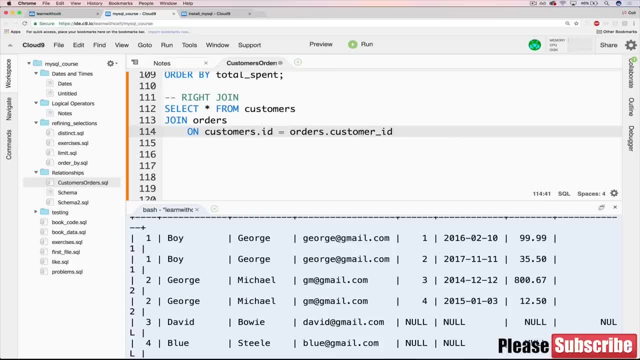 orders dot customer ID, just like that. However, if we leave it like this, remember, if we don't have a matching record, we're going to have a matching record, So we're going to do a right join, And if we don't explicitly say what type of join, it's implied. 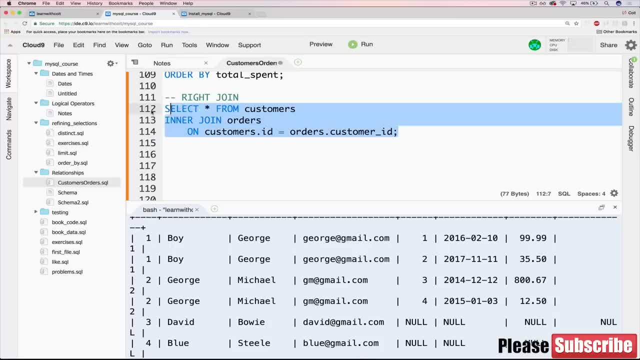 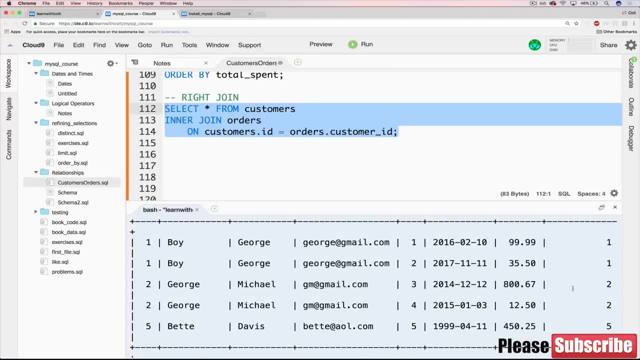 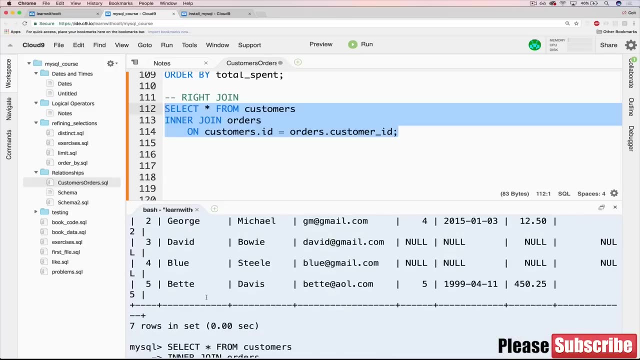 to be an inner join. So we can actually start with that, because it will be good to see what that looks like and compare it to what we get when we do a right join, So when we did left, which is right here, we have these nulls And we have, let's see, 1234567 entries Versus. 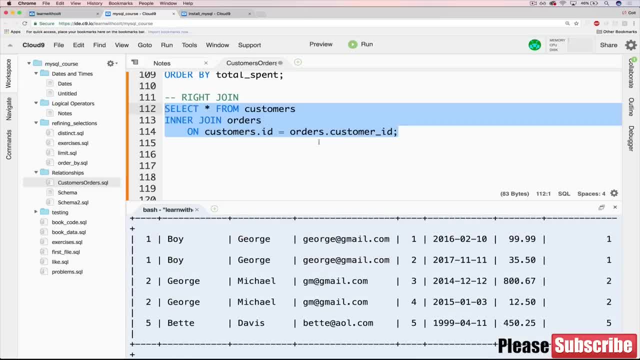 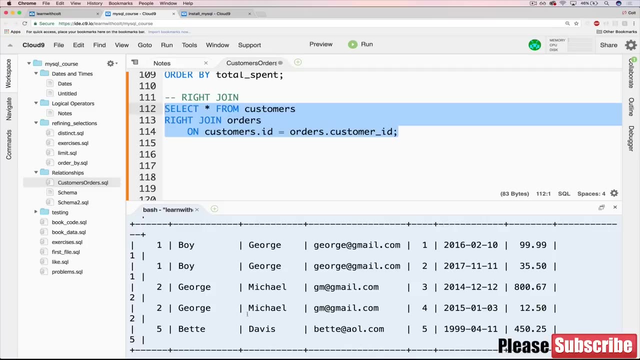 when we do an inner join, we have five, And if we make it a right join, all we have to do is change that. If I can type right, there we go, Let's try this one, And we have five again: 12345.. And. 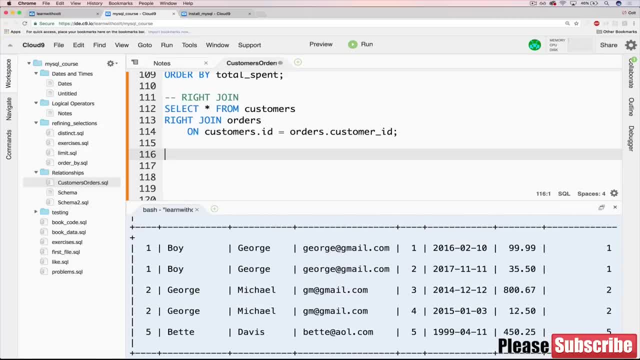 actually it's identical to what we got when we did the inner join, And the reason that's happening- I kind of already went over this briefly- But the reason it's happening- is that we don't have any orders that don't have a match with a customer. So everything we 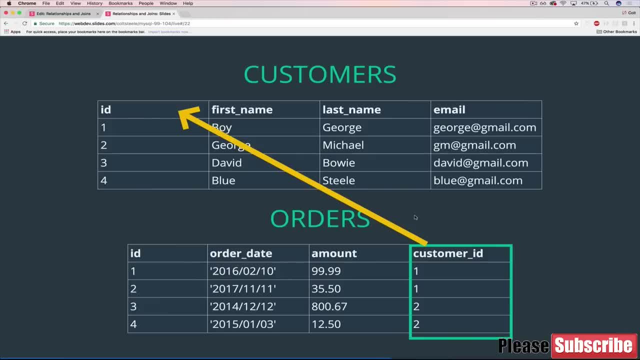 have. if we go back here, everything we have in the orders table has a matching customer, So there is something to join it on. So for every order we actually have five- this table only has four, but we have five in our database- then there's only going to be five joins when we are just going. 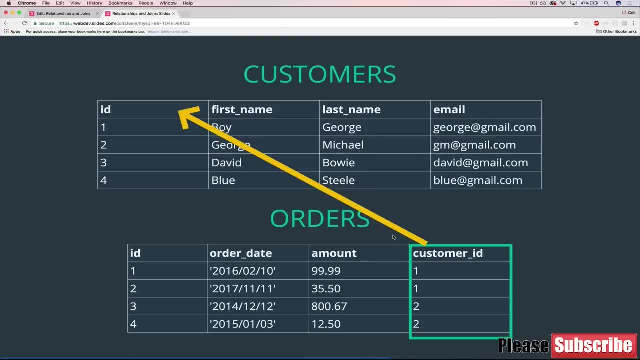 to be five records that are joined When we do a right, join when we did a left. we had a bunch of- well, not a bunch. we had a couple of users who didn't have any records, didn't have any orders. So we use customers like David Bowie and Blue Steel. So we have a couple of users who 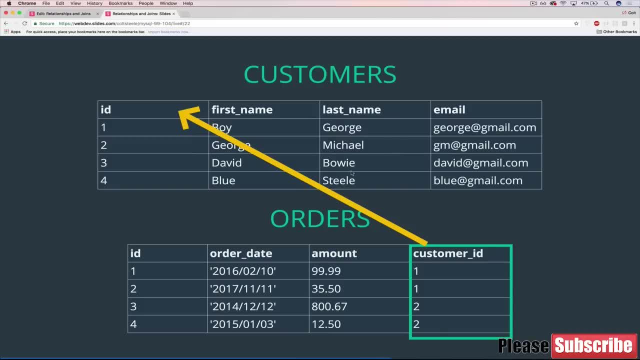 didn't have any records, didn't have any orders. So we have customers like David Bowie and loose steel didn't have a match, but we still included them. So how can we actually see something different? How can we tweak our data so that a right join actually results in something distinct? 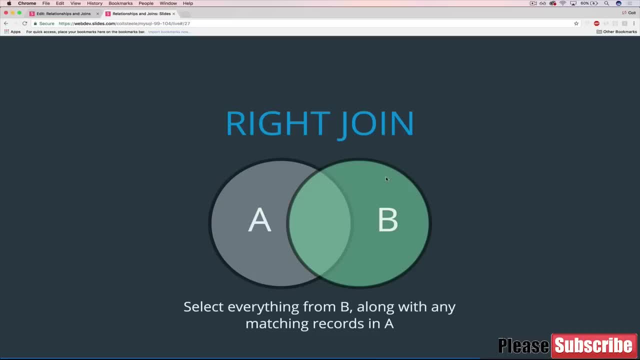 Well, there's a simple thing we can do, which is to screw with our data or, excuse me, to mess with our data. So that's what I'm going to do here. I don't necessarily recommend that you follow along exactly because I'm going to be messing up some of the data. I'll fix it towards the end of the. 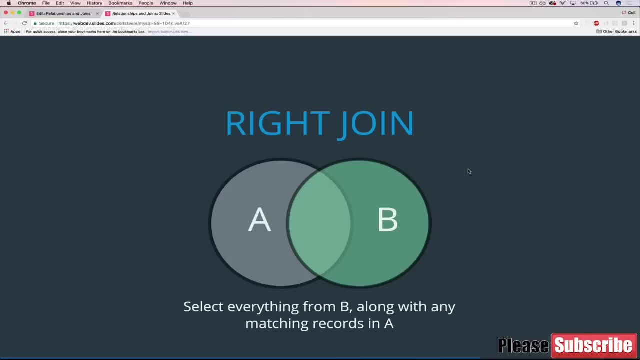 video, but I don't want you to have to go through that process if you don't want to. So it's not essential. What is essential is how the join will work which we'll get to. So the way that we would have a difference, we'd have a unique result between right and inner, is if there's something. 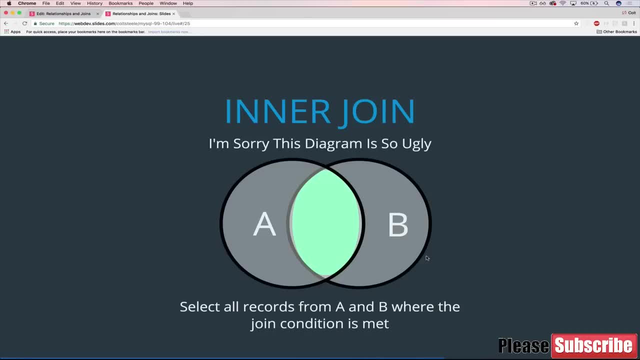 that we have on the right table, which for us has been orders In the orders table. if there's something in the orders table that doesn't have a match over on the left, there's no join, So that would mean that there's no customer. 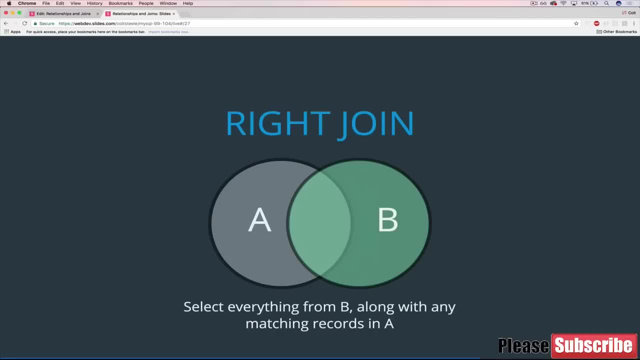 And right now it doesn't make sense, honestly, to have an order without a customer. But maybe, let's say, someone accidentally deleted stuff from our database Or maybe there's a wrong ID, a wrong customer ID, in our data. We would be able to spot that using a right join. So what I'm going? 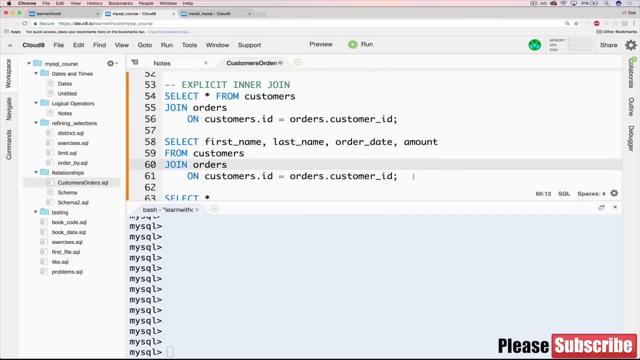 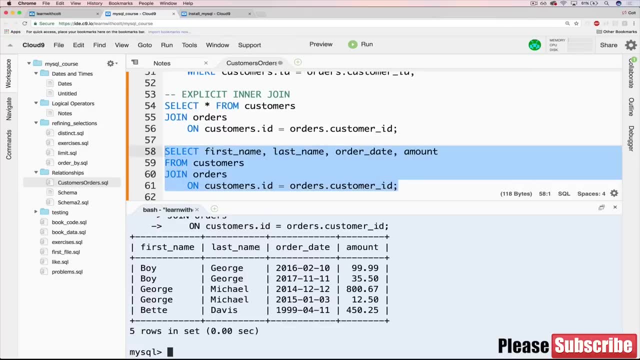 to do is hop back to Cloud9. And before I do anything, I'm just going to rerun this early to let you guys know just the inner join we did. So, as we can see, of course, on the left we have. 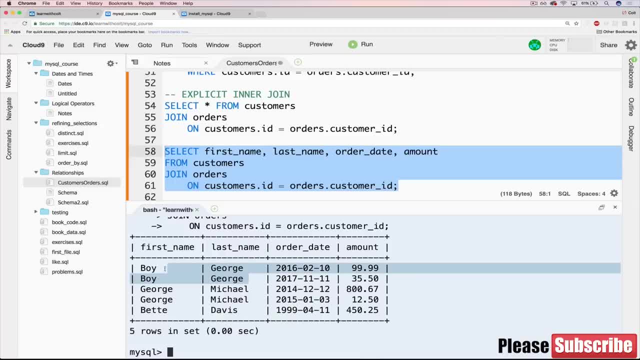 customers On the right. we have orders And we have Boy George who has two. Let's say I were to delete Boy George And then I ran an inner join. Well, these would be gone And we would only have three customer orders. But if I did a right join we would have order, order and null and null over. 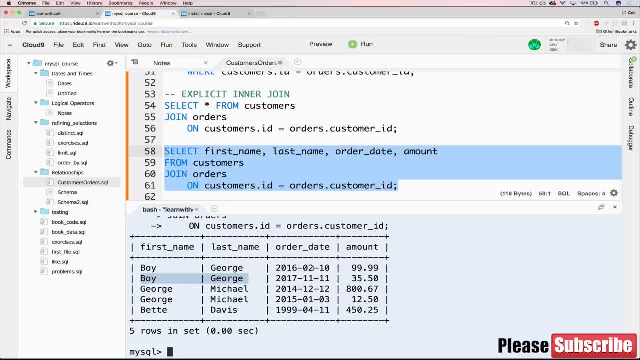 here, here. so it takes all orders, regardless as to whether they have a matching customer or not, and they'll fill in null if there isn't a customer, and then, if there is, the appropriate information will be filled in, just like it was with left, except you know the opposite direction. so let's try that. let's try. 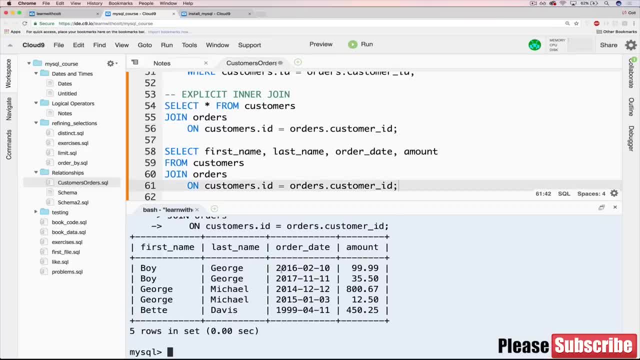 deleting a user or a customer. let's delete boy George. it's been a while, but that's going to be delete from customers that keep calling it users where? and we could do it based off of ID, let's do it based off of first name, first name. 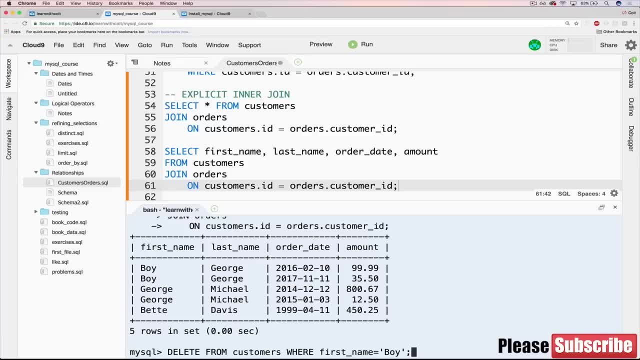 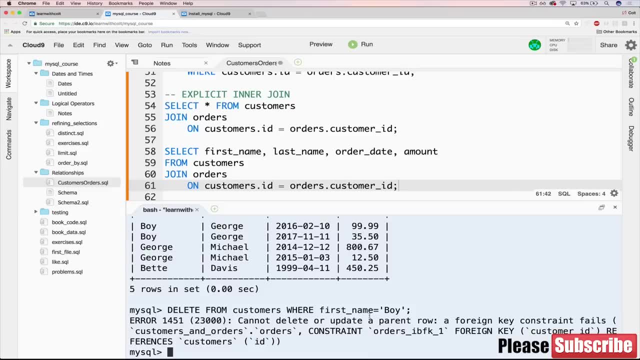 equals boy, just like that. now what do you think will happen? oh, no, an error, and you may have anticipated it being a syntax error based off of my typing proficiency, but it's not. it's an a deeper error. it's an error that has to do with that foreign key constraint we set up, because if we try and delete a 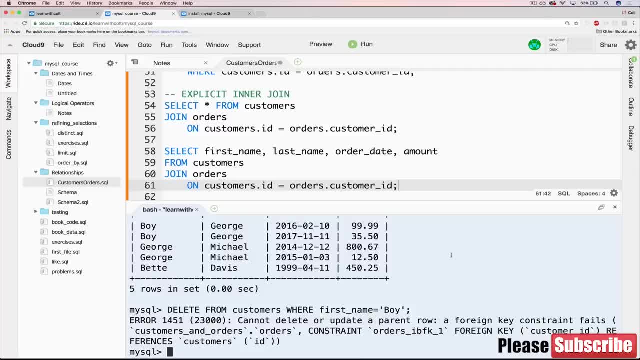 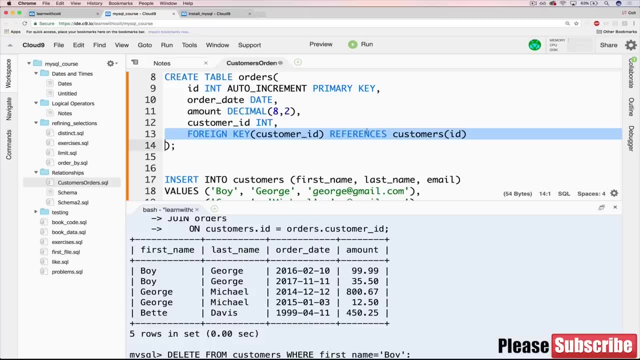 customer that an order is referencing. we have two orders referencing. we have two orders referencing. we have two orders referencing it. that's a problem according to our foreign key constraint that we set up up here. remember that this doesn't let us create an order with a faulty or 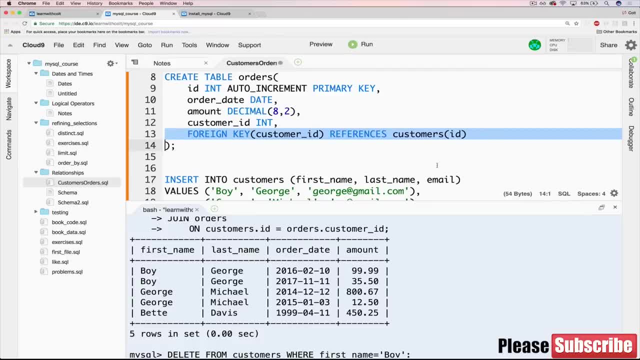 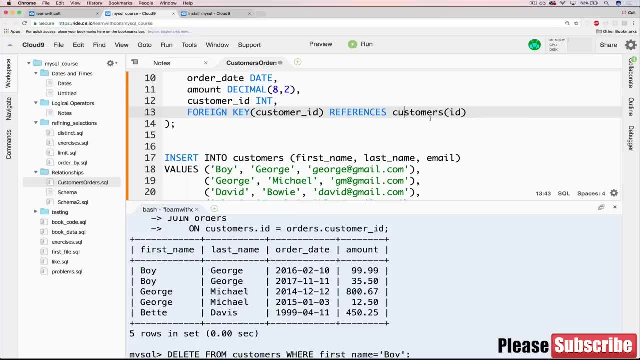 non-existent customer ID. so it also won't let us delete a customer up here if it's dependent on down here. and I kind of did this on purpose here to show you a solution to this, not to let us delete things willy-nilly, but how could? 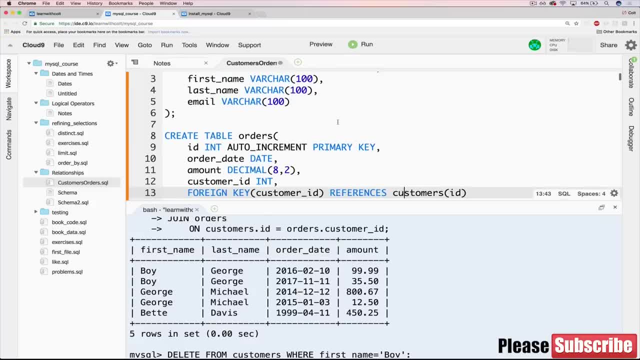 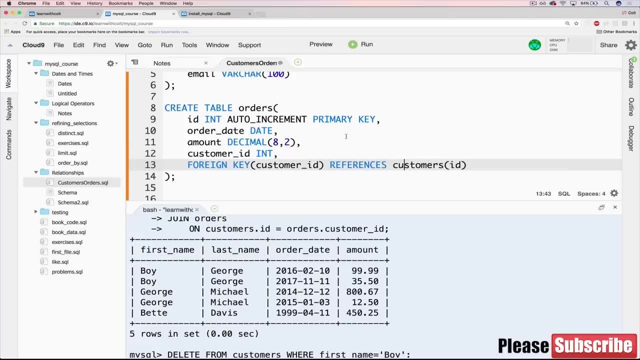 we. if we deleted a customer, how could we automatically have it delete all orders associated with it, which is a pretty common thing if you have data that's dependent on another piece of data. let's say we have books and reviews. well, if that book is deleted for some reason, we don't want all these reviews. 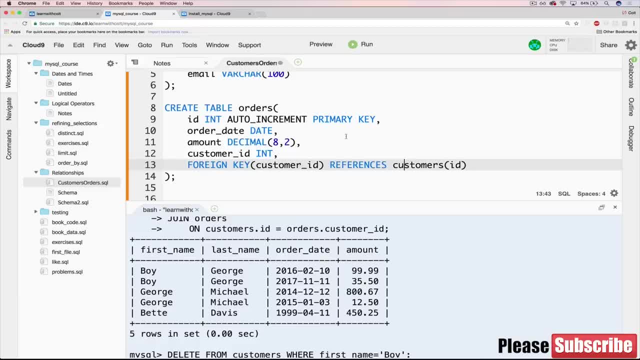 that are just pointing to an empty or gone book, so we would want to link them. so if I delete the book, all associated reviews get deleted, and I'll show you how to do that. but the first thing I'm going to do is delete these two tables. 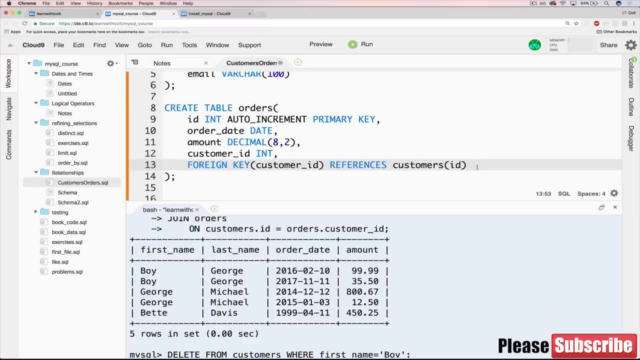 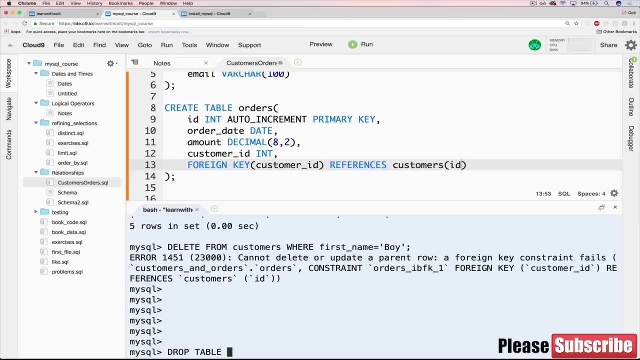 I'm going to remake them, and this is the first thing I'm going to do is delete these two tables. I'm going to remake them, and this is the part I was saying. you do not need to follow along, so let's do that now. drop table, and we have another little surprise in store for us if we try and 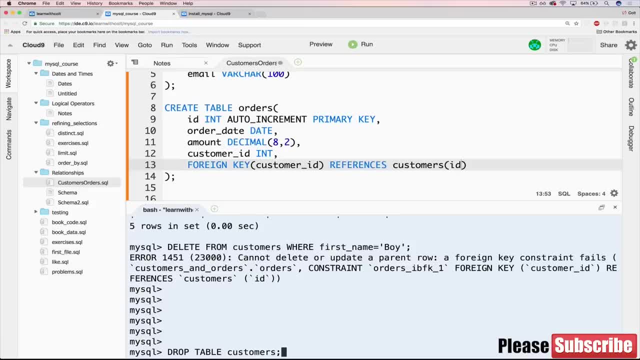 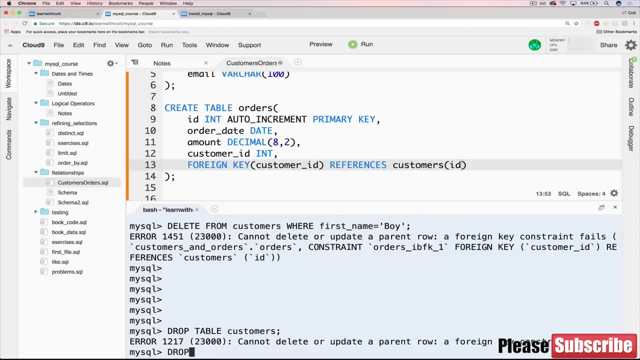 drop table and let's just do customers, what do you think will happen? same issue: we can't delete customers because orders depends on it. so what we can do is delete orders first and then customers, or we can do it in one line like this: orders comma- customers. well, if I put the order first and then we get the order, 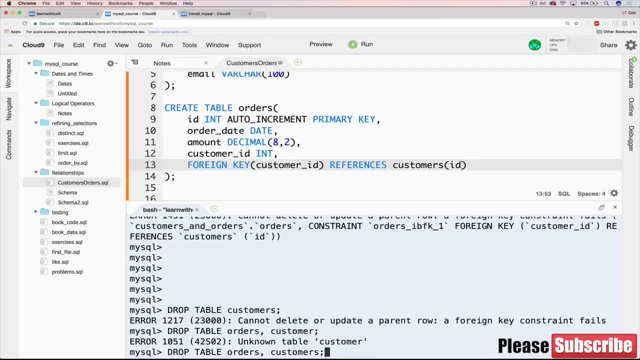 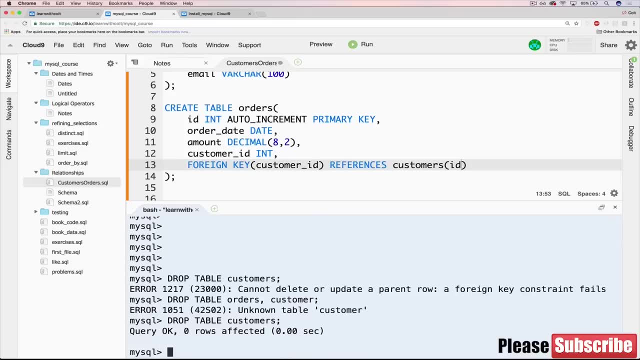 orders, comma customers. well, if I put the order first and then we get the order, put an s there and now of course i messed it up because orders is already gone. so if i had typed that correctly it would have worked. but we'll just delete customers separately. now, if i do show tables. 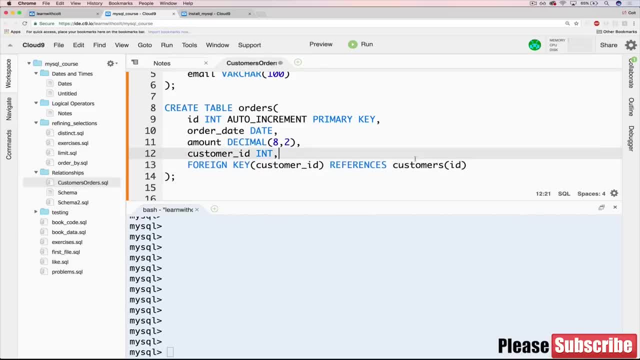 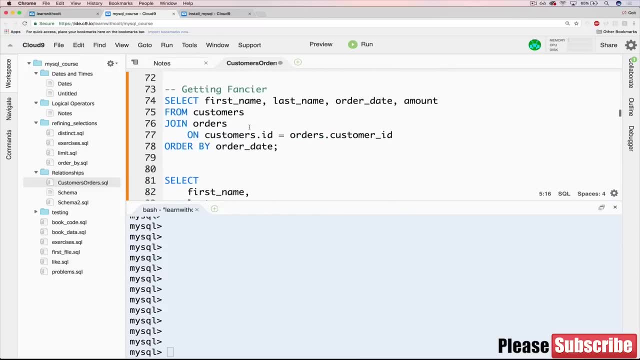 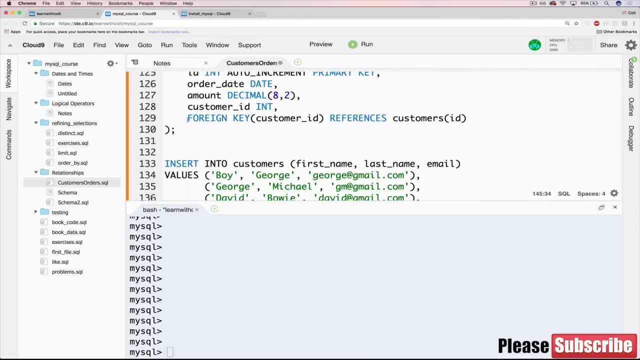 there's nothing there, okay. so the reason i did that is i want to remake our two tables, very simply. so i'm going to copy this and this is why i was saying you do not need to do this yourself, necessarily, and i'm going to change one line. i'm going to get rid of the foreign key. 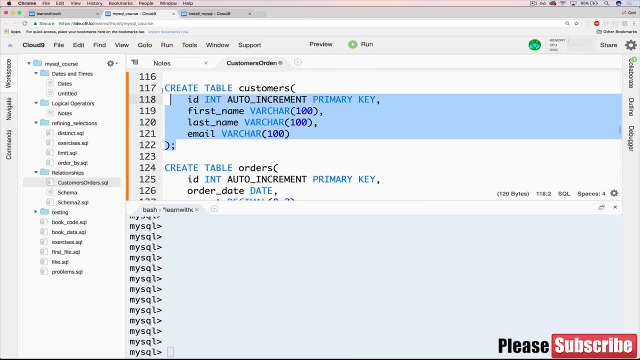 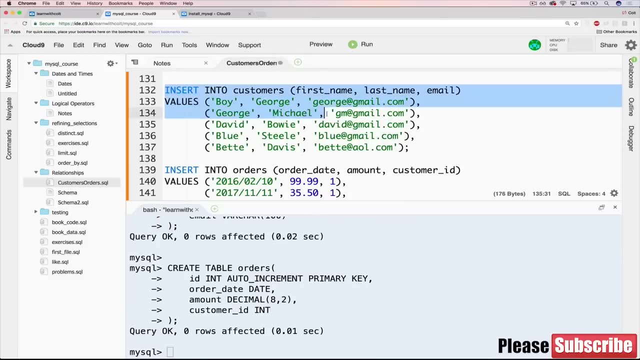 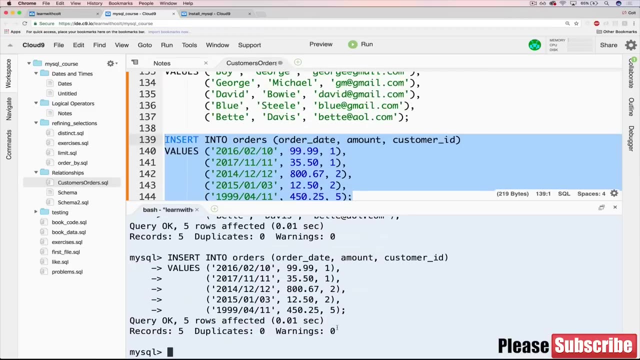 constraint, just like that. everything else should work exactly the same. so i'm going to remake the customers table, remake the orders table. i'm going to insert our customers and i'm going to insert our orders, just like this. okay, so if we do a select star from customers, let's say 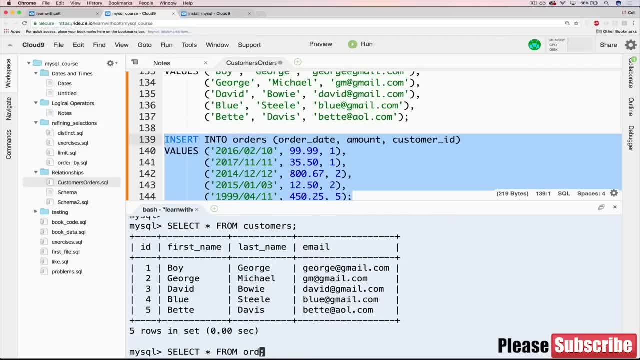 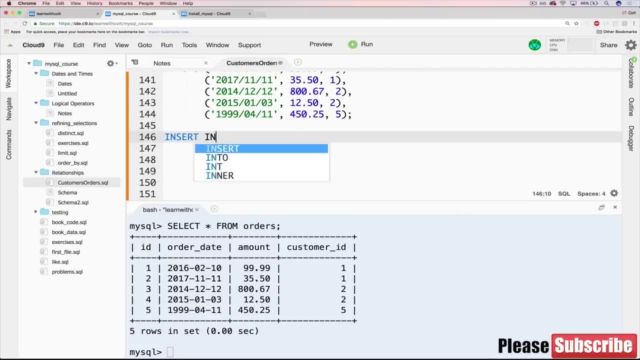 we have the same data, you same thing, from orders. but now what i'm going to do- is i couldn't do before- is i'm going to insert a new order. so insert into orders and i'm going to insert what do we have: order date, amount and customer id. and i'll do two of them, and so the first one. 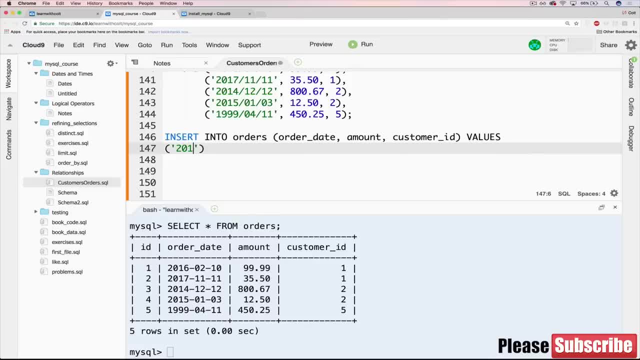 will be something ordered, let's say, 2017, slash uh, i'll 11, slash 05, and the amount was 23.45, and the customer id. this is the important part that i'm trying to highlight here. i'm going to put something in that doesn't exist in our table. 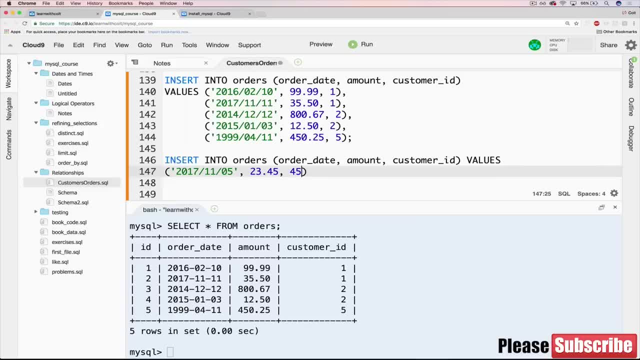 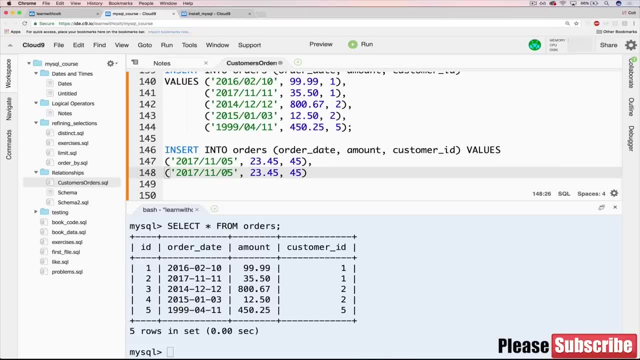 so let's say 45 and i'll do one more i'll do rather than this. let's get a little practice. remember, using cur date gives us the current date. let's do that, so we'll do cur date here. comma. and this purchase was for 7077, 777.77, and that was made by someone with id 109, which also doesn't exist. perfect, so. 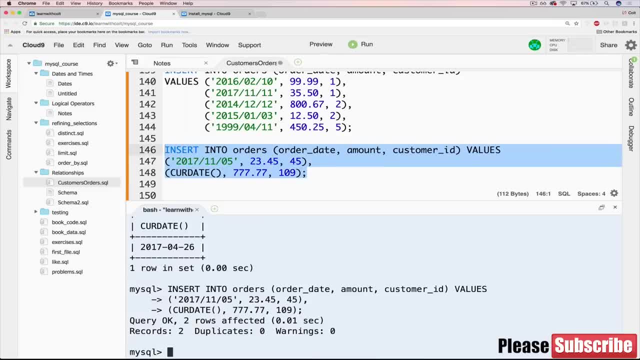 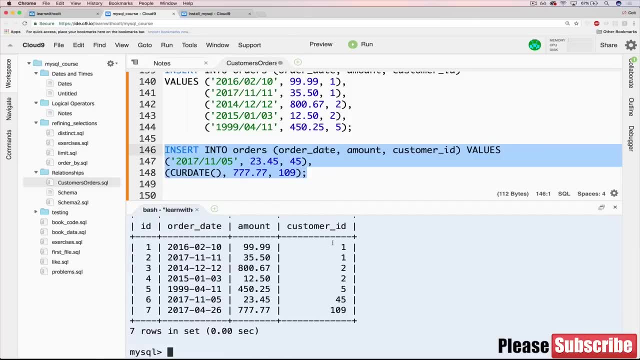 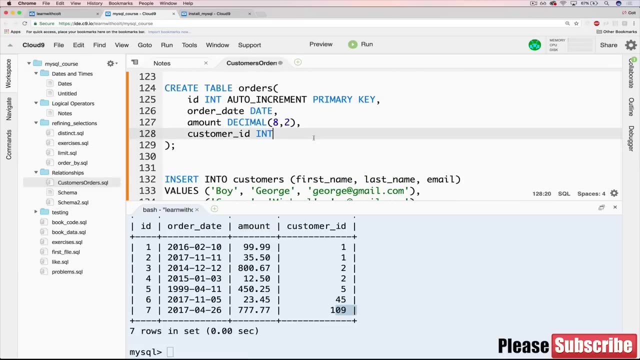 now let's insert those. didn't seem to have any problems. let's look at orders. yeah, it's here. right, we have customer id of 45 and 109, and the reason this works is we got rid of that foreign key constraint, which i'm not saying you should do, by the way. i'm doing this. 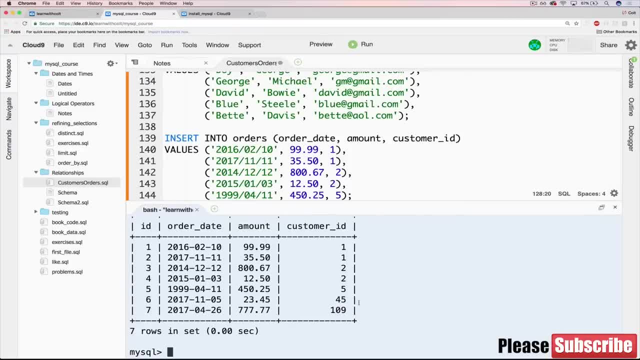 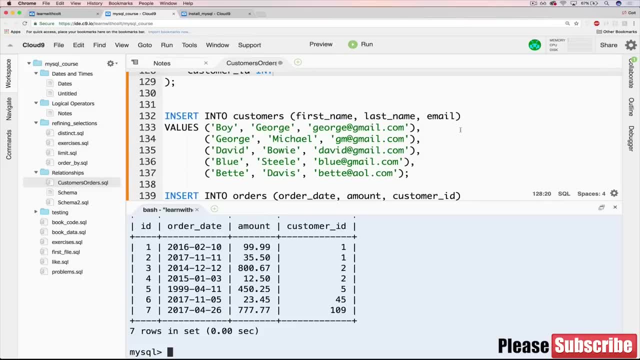 to illustrate uh and make a difference in our data. so let's suppose we're inheriting someone else's database and they decided not to use foreign. they didn't know about foreign key constraints, so they didn't use it. and then they had users they used to have all the way up until 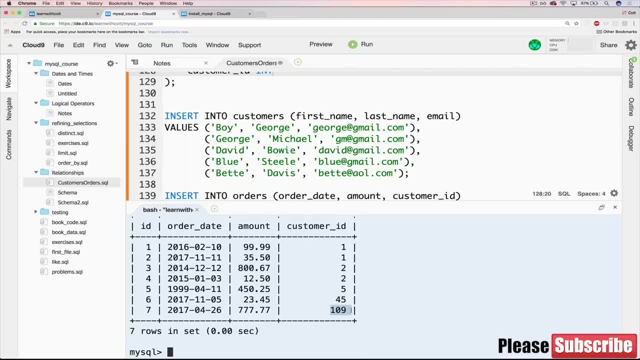 109 users or customers, and then a lot of people left. they just deleted their accounts. let's say, something bad happened. there was a hack, a data breach. everyone got scared away and then all we are left with are these customers. it's pretty sad, so what i mean? it's a great bunch of customers to have. honestly. 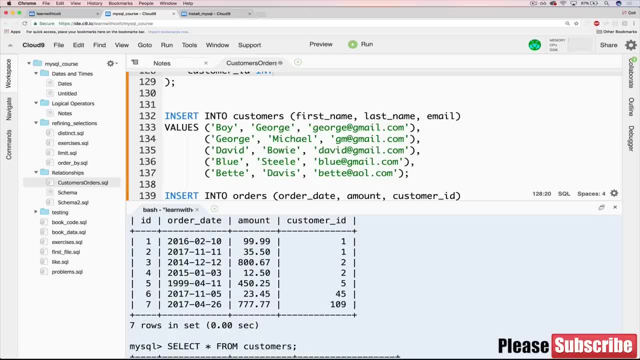 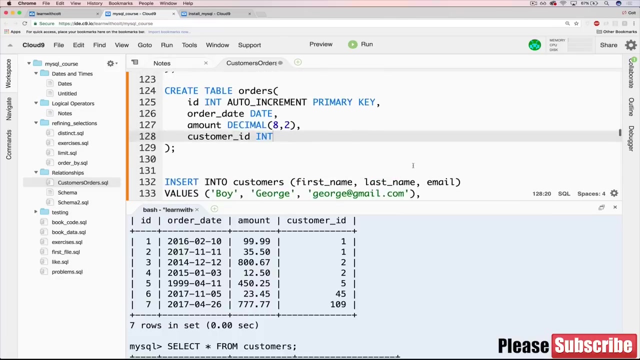 but still only five compared to 109. keep in mind, this is all a dumb made-up story, but what we could do is use a right join to basically identify, uh, all of our customer and orders and their associated orders, as well as any orders that don't have an associated customer, so we could fill in null. so, if we do our join, that we had done. 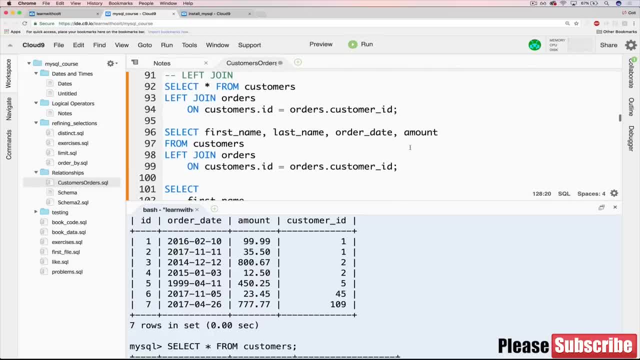 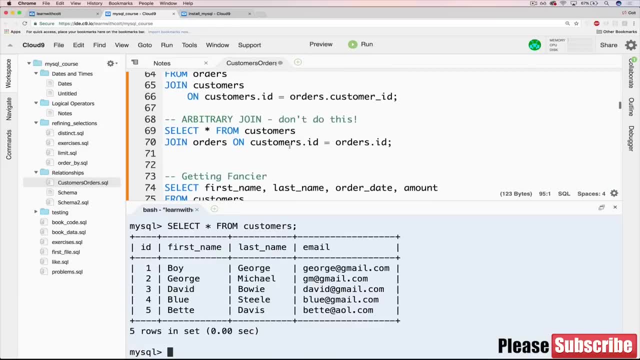 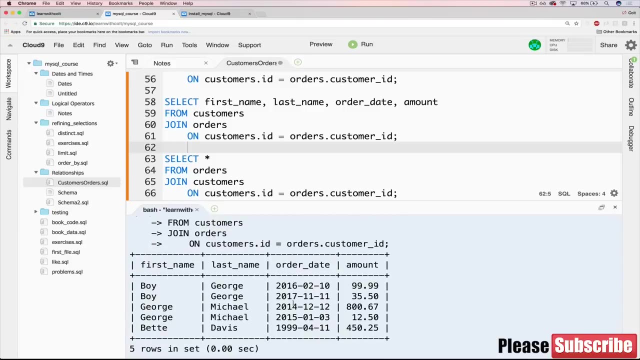 earlier. i'm just going to scroll up to save times, or save time, if we do this join here, which is an inner join, or that's actually a left join, let's do this one right here. nothing changes, right? we still have boy george and his associated uh, two orders george, michael. 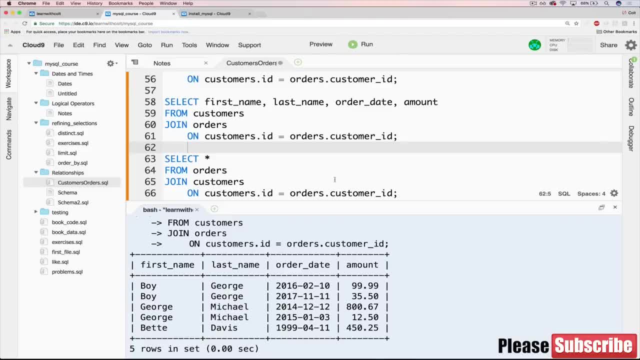 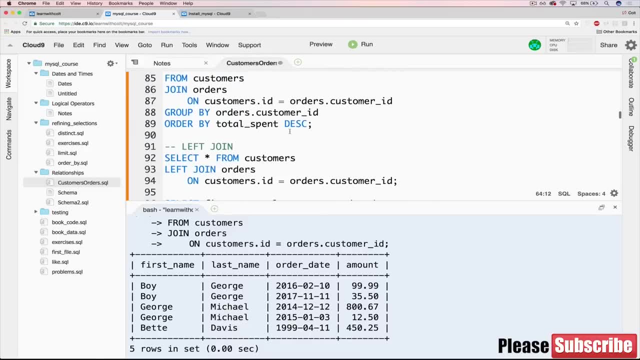 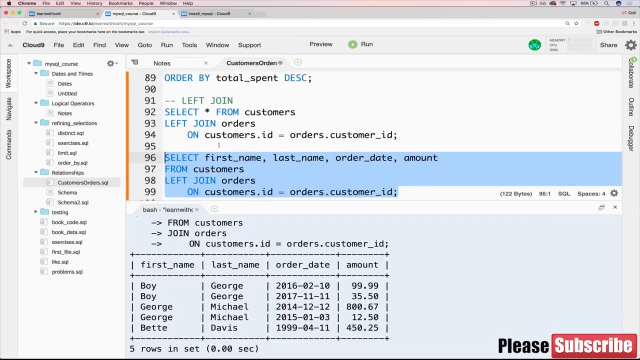 his two orders, betty davis, her one order, and then if i did a left join, which we could just do by simply changing that one, uh, inner, to be left, or we can just do this here, and i'm only choosing this one because, rather than star, this has a smaller subset of data that's easier to look at, okay, so 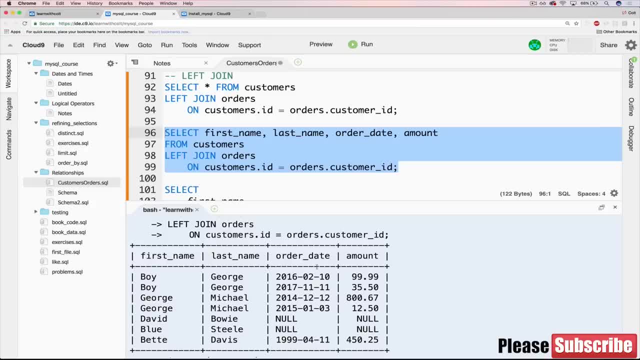 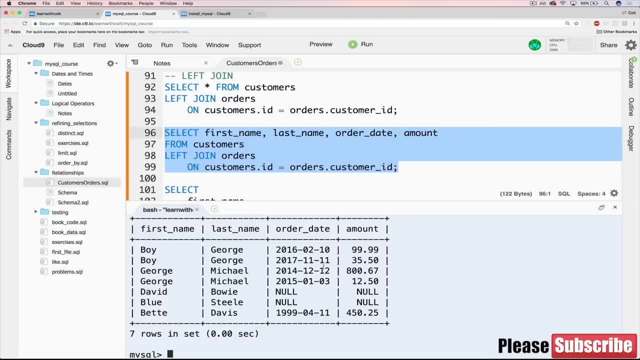 now we end up with this, which still is unchanged from when we did it in the last video, because there are orders that have no customers but they're not here, because we did a left join and the left join takes everything from customers and any associated matching data from orders. 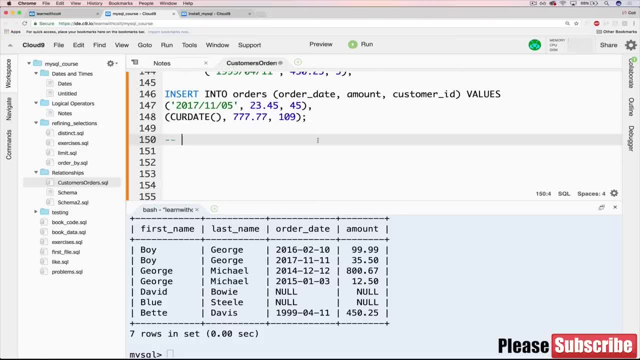 but now if we do the same thing down here- if you can hear my cat meowing- and we just change it to be right, join. so we're still just doing first name, last name, order, date and amount. so we are SRAM right. join, also in review if we go down from customers on the left. 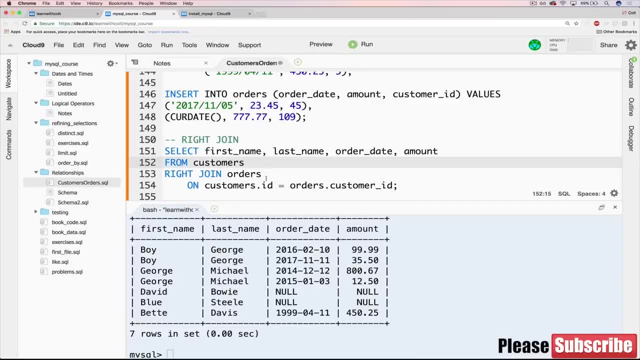 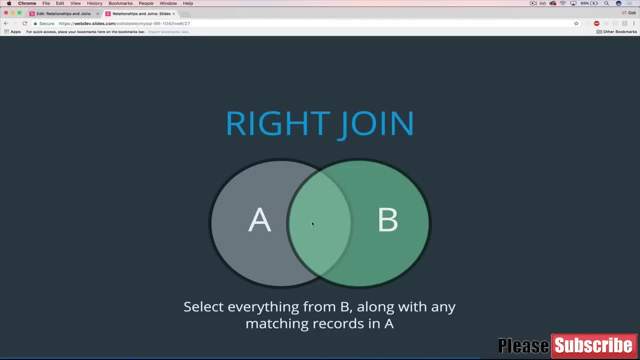 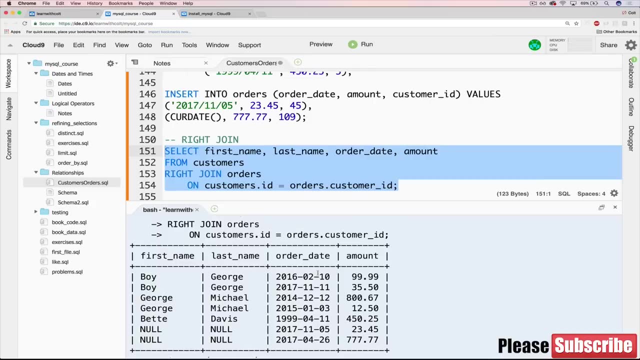 or from on the left is wrong term, but From Customers. First write Join with Orders So that we take everything from orders like this, everything from orders in any overlap from customers. let's try it and you can see exactly what we expected happened. so we still have all of our orders that match. 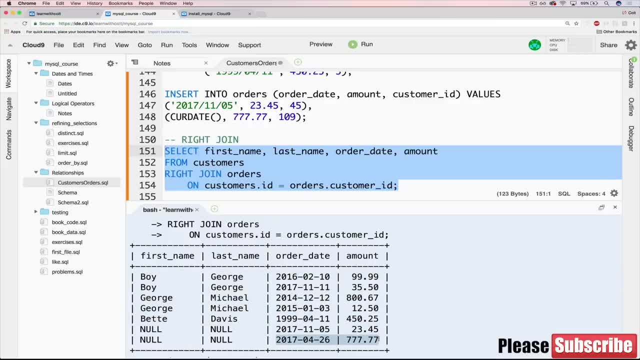 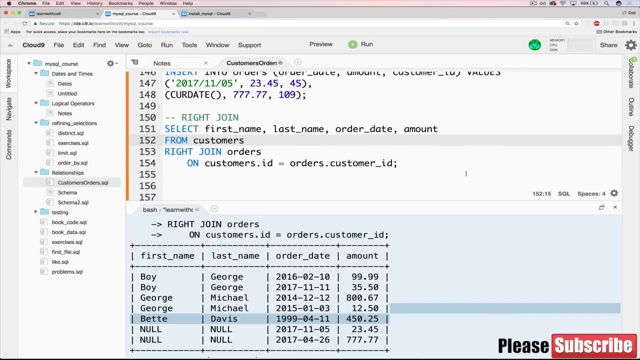 customers and orders added in where there is no matching customer. so we end up with null first name, null last name, null first name, null last name. so that's basically all i wanted to show you with right joins. but, like i said, we will have actually relevant, useful examples later. but the last thing i wanted to do 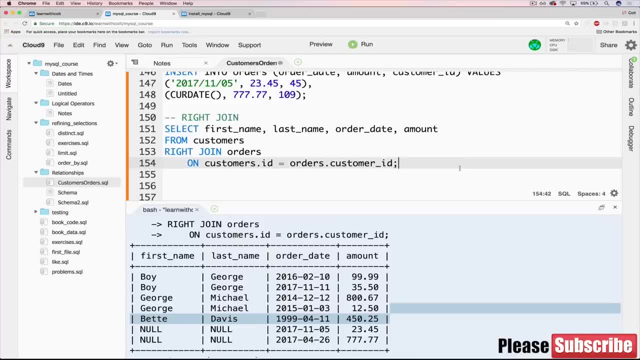 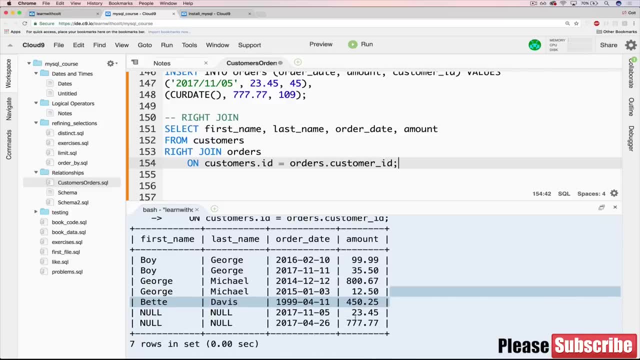 was hit you with a whole bunch of setup, brand new data, just so that you could see how a right join works. so there is. you know, this is a hypothetical situation that could happen. we could have orphan data like this. so i'm going to show you two things now. the first one is that we can still just do any. 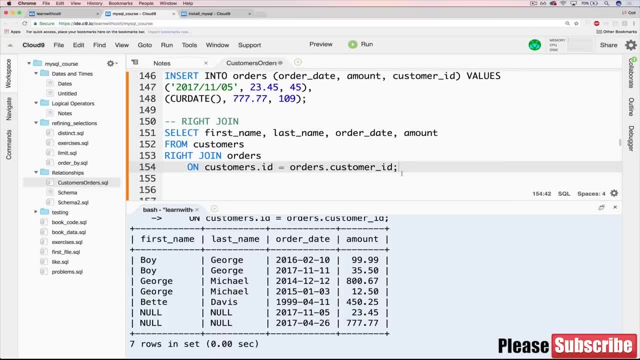 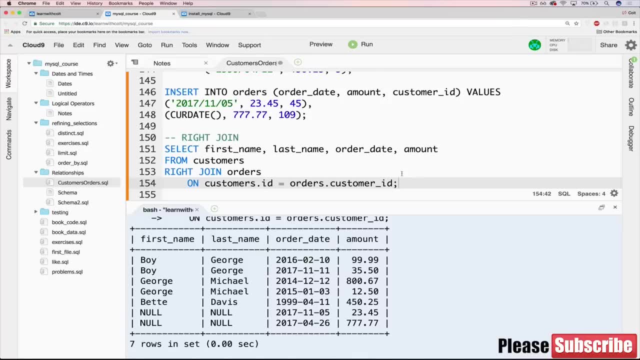 you know anything that we want with this data. like we did earlier, we can do more complex selections, and i'm also going to show you a new constraint you can add to your schema so that when something is deleted that has a foreign key depending on it, it will automatically delete the dependent record. 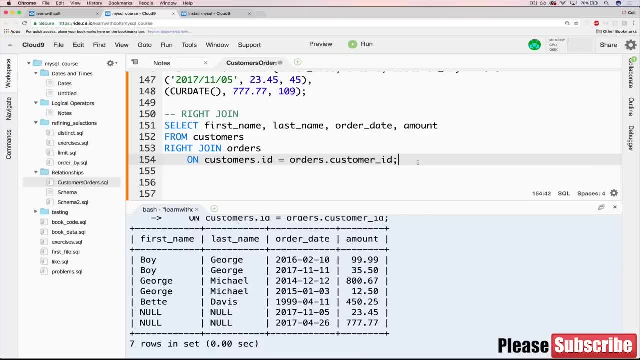 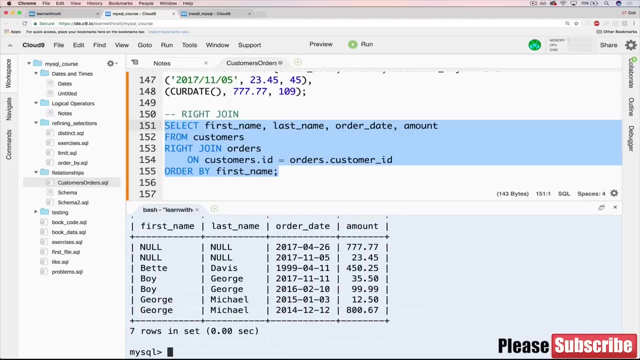 but to start, i just wanted to show we can still do things like group by or we can do things like order by. so we can add that in here. let's do order by and let's do first name, just like that. okay, what about if we tried to group by? what if we did group by? 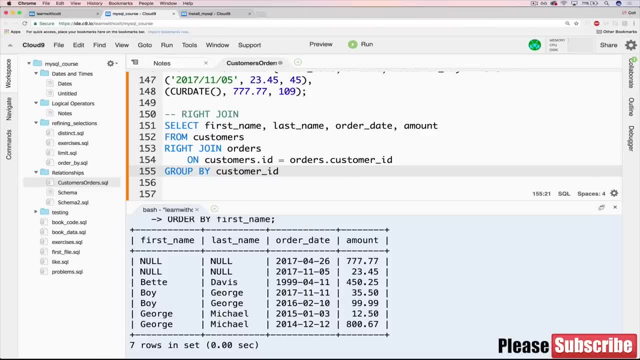 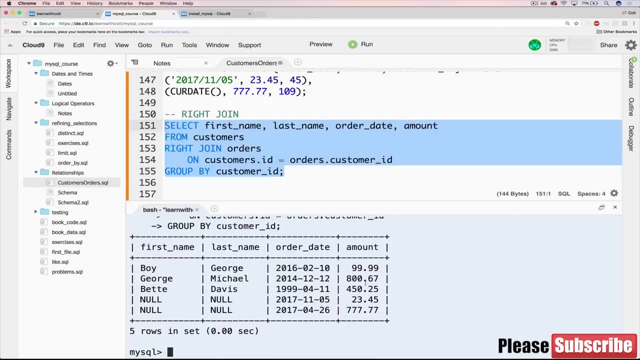 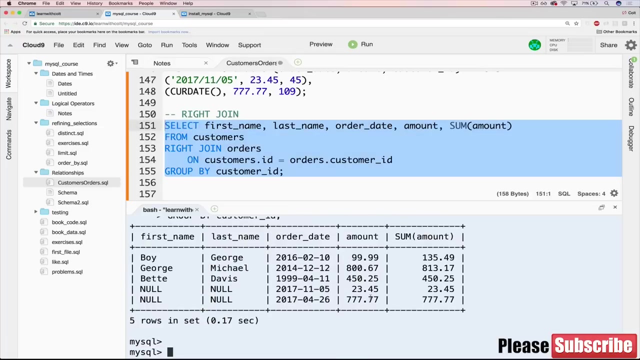 and what if we tried to group by customer id? what happens then? so it doesn't look like all that much, right, um? but we can still do our same. you know, we have boy george was condensed, george michael condensed. but we can do a sum for amount, just like we've been doing, and we can see how much everyone has. 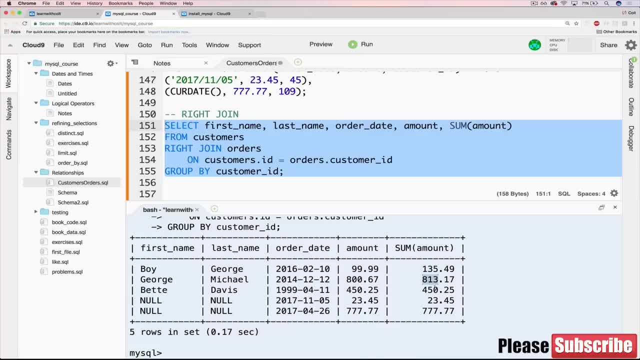 spent boy george: 135. george michael: 813. betty davis: 450.. we still have these two nulls, so this is where we can start to make decisions and do things like: okay, if first name is null, then let's replace it with something. 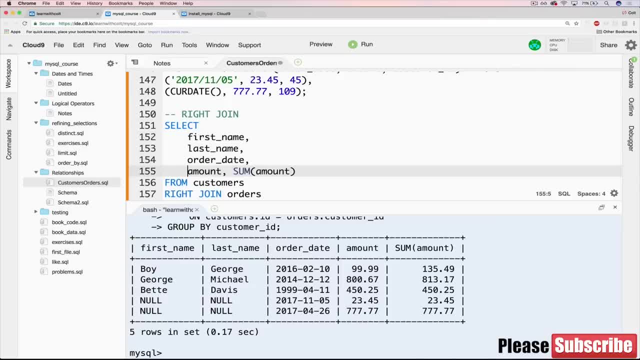 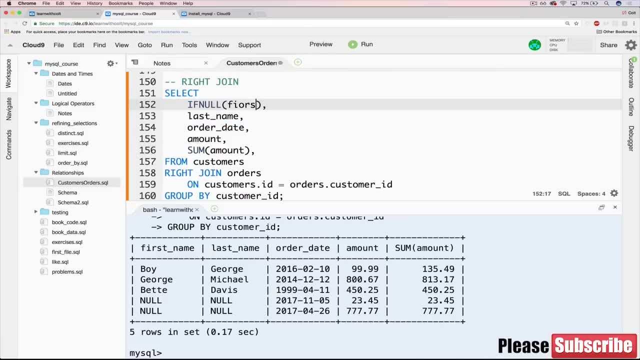 so i'm going to format this a bit as we start to get more and more and we'll replace first name and last name with, if null first name, and remember how this works. if first name is null, then it will be replaced with whatever we pass in. so we'll say we'll just say missing. 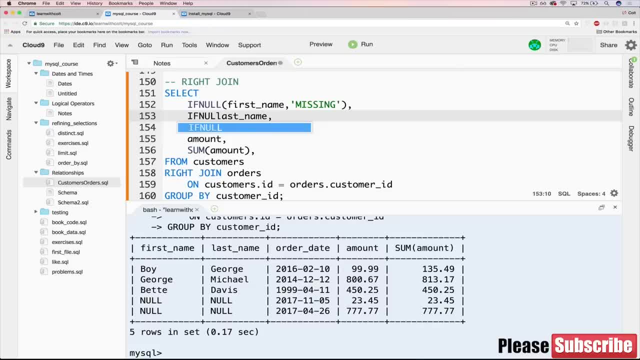 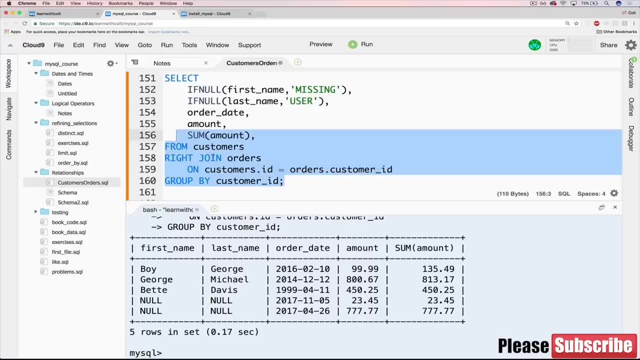 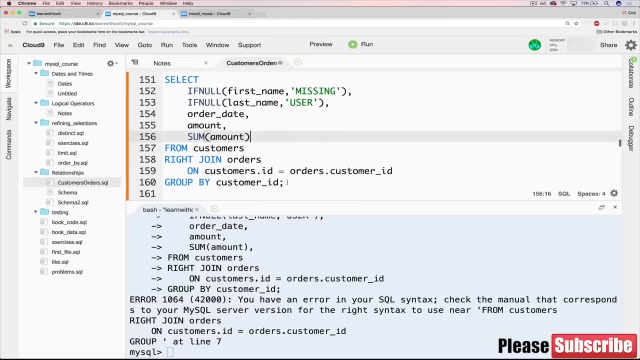 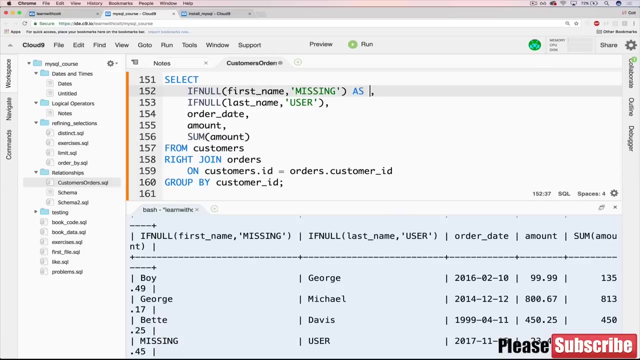 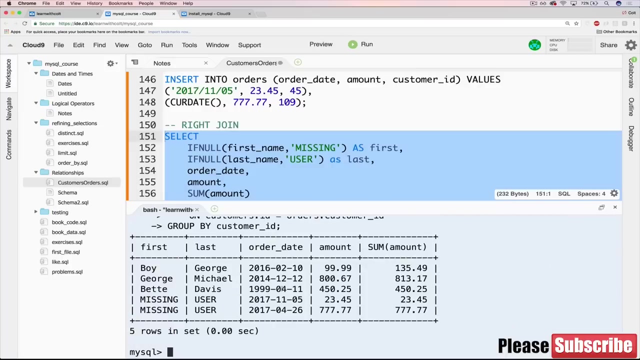 and then we can do the same thing for last name. if null last name comma, we'll say user, so we'll end up with missing user. if we do it that way, if we don't have an error or extra comma here, now we do it and let's use aliases as first as last. all right, got a lot going on, okay, so now we have missing. 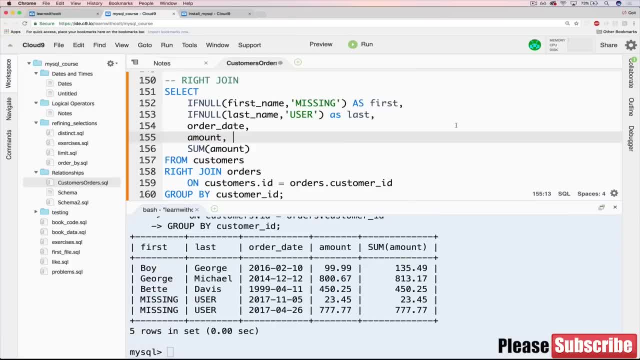 user. and let's say we want to see what does this look like. so let's say we want to see what does this look like. total of our orders are where we don't have a user. so basically the orphans. we want to group those together as well. right now we're grouping by customer id, but what if i wanted to group these? 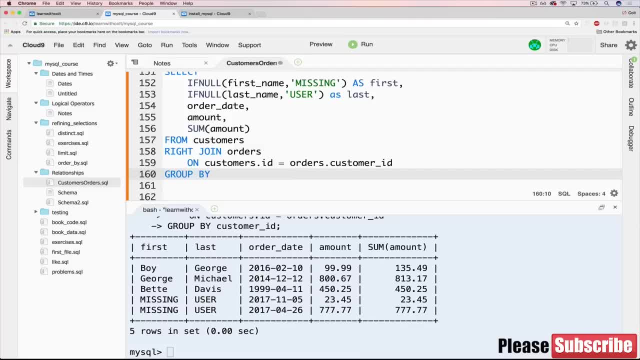 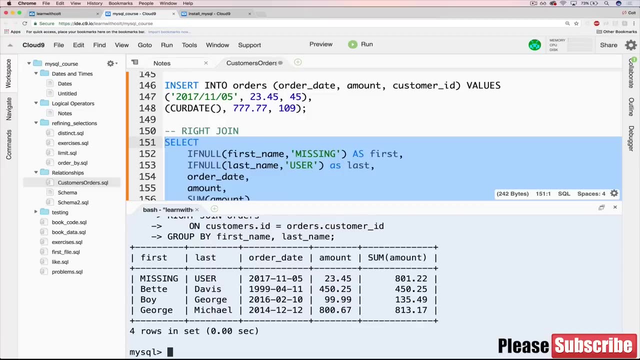 two, what we could do is change customer id to be first name, and we'd want to do comma last name rather than just first name, because we may have multiple people with the same first name. so if we do this now, you'll see that we end up with missing user has 801 total spent, then betty davis 450 and so on, and 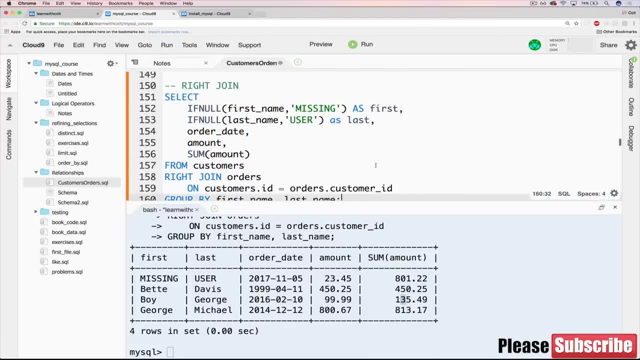 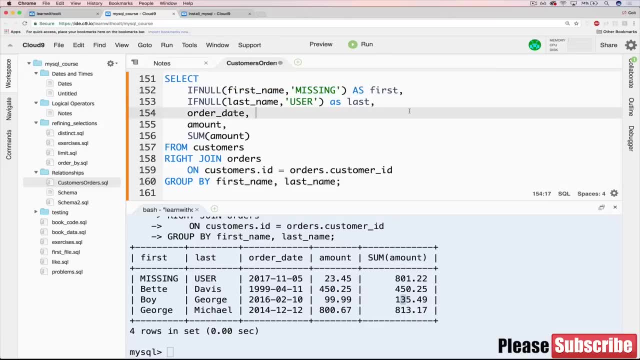 we could order it. i think by now you understand what i'm trying to show, that these tables aren't special. uh, you just have to be comfortable working with null and if null is kind of your best friend when you're doing that, okay. so then the very last thing i wanted to show: 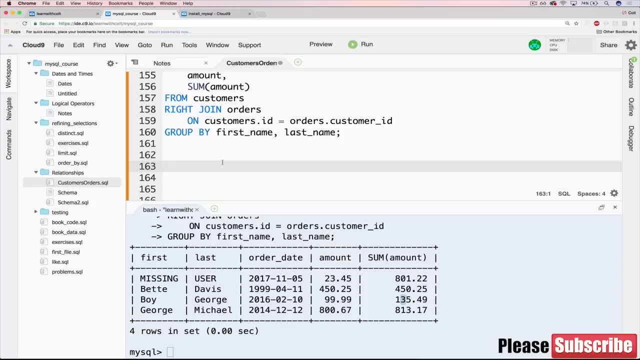 keep doing that, go away. the last thing i wanted to show was how we do what's known as on delete cascade. so this is what i was talking about: when we delete, if we have a foreign key relationship, when we delete a parent. so if we delete customers table, not the whole table, but 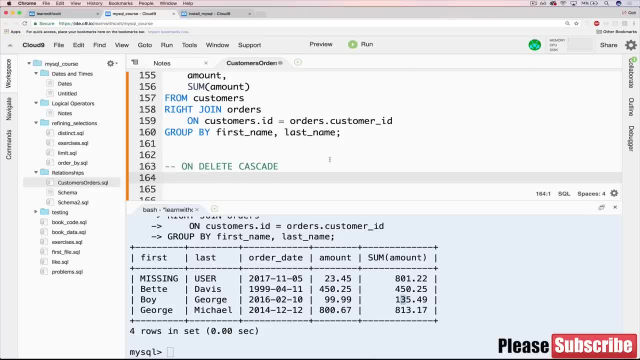 let's say, we delete betty davis, we want her order to also be deleted, so it's not just totally on its own. we don't end up with this situation. so how do we do that? well, i'll show you right now. if you're not interested, then go ahead and skip. this is. this isn't about joins, but i figured it. 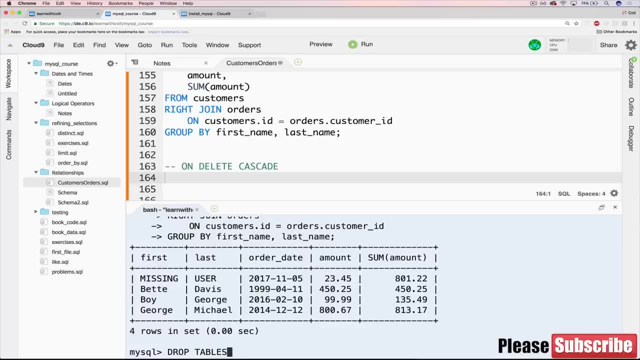 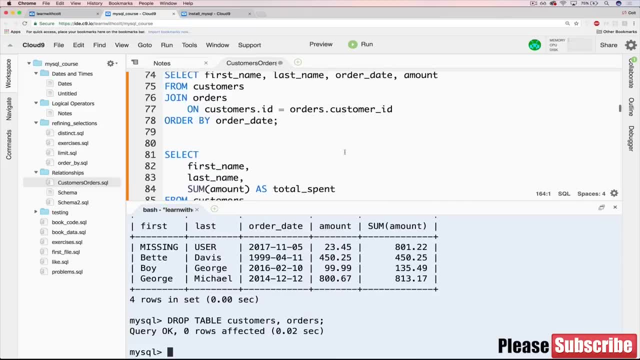 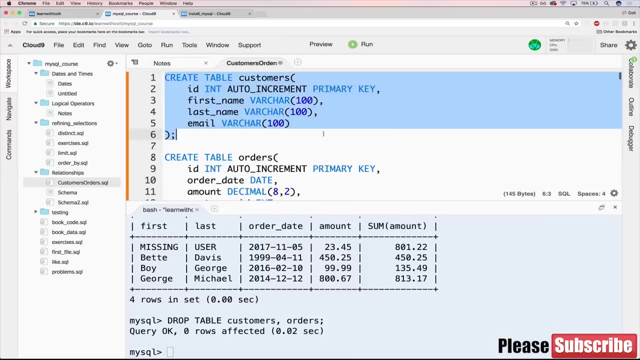 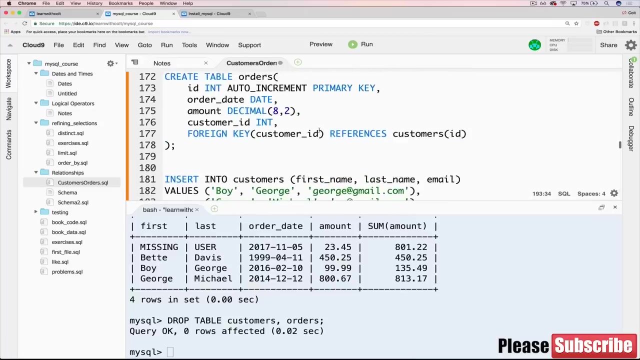 is a good place to put it. i'm going to actually drop our tables again. i'm going to redo, so grab our original schema from way up here, just copy how much do we want down to here, and we still have our foreign key there. i'm going to indent this a bit. 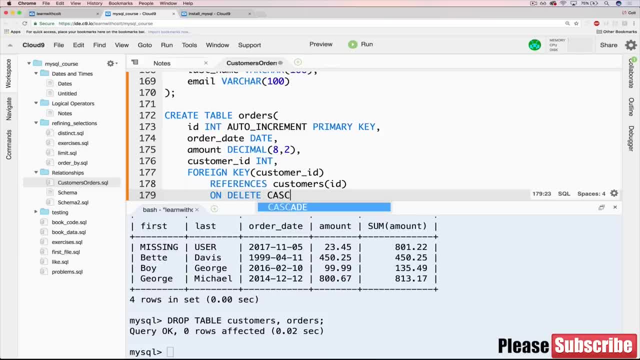 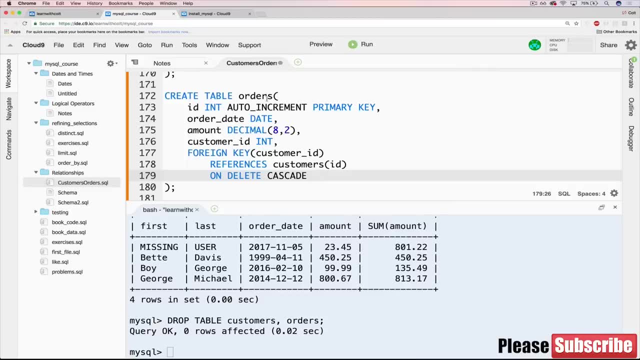 and all we do is add on, delete, cascade, and all that that does is it says: when a customer is deleted that has a corresponding order, delete the order as well. So let's try it. I'm going to copy this in: Let's make sure we don't have any tables right now. Perfect, So let's copy it. 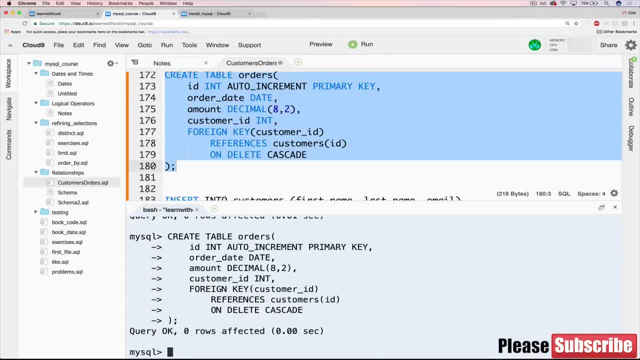 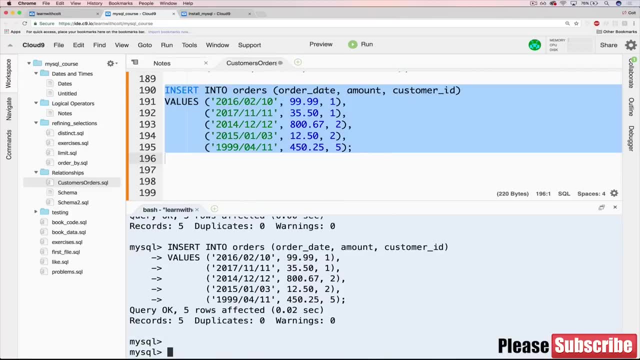 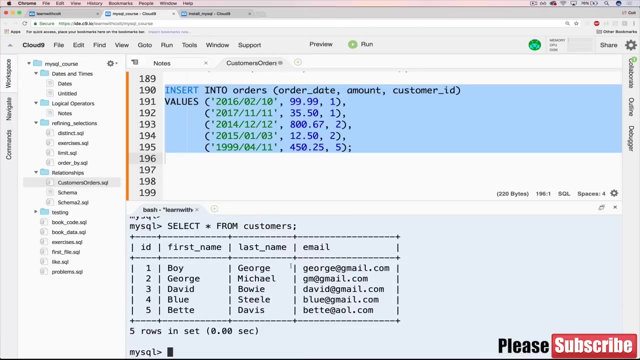 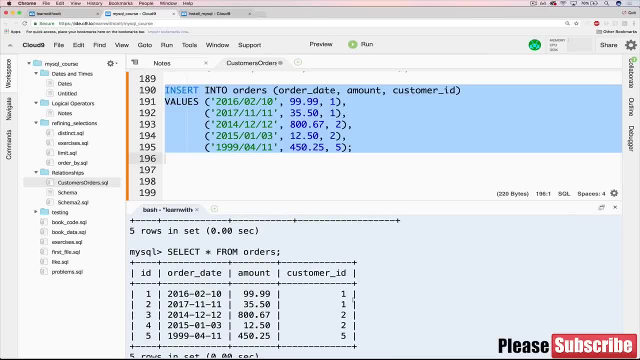 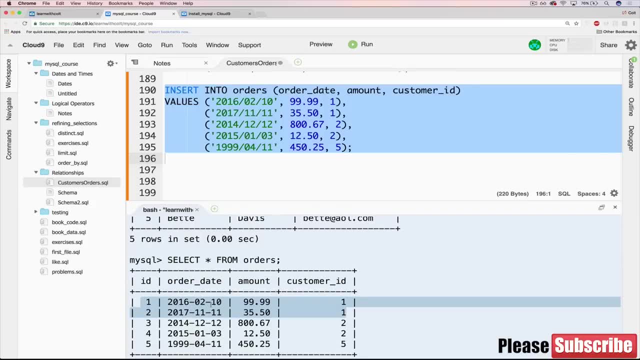 Let's delete boy George. Boy George has two orders, These first two. So if I delete boy George, these two should now disappear versus in before a couple minutes ago, and we tried it, we had a problem. It's not really a problem, but we we ran into trouble that we put in there. 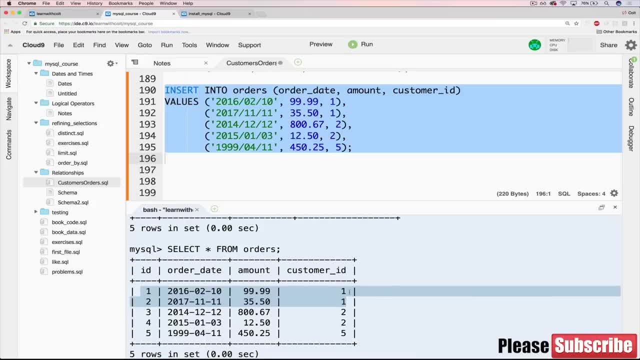 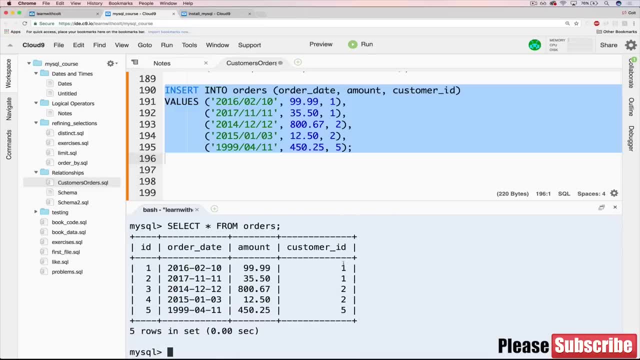 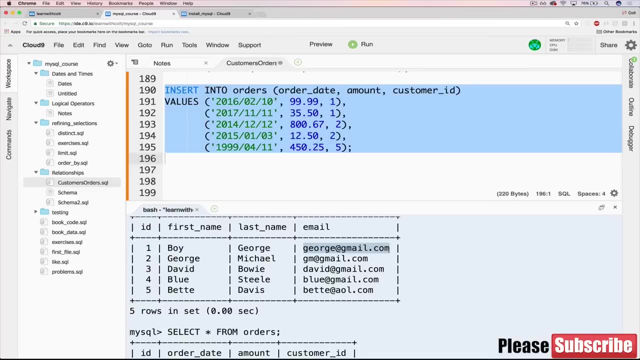 ourselves because the foreign key constraint didn't allow us to delete it. We weren't allowed to delete a customer unless we deleted the order first. So we're going to do that now. Just try deleting based off of ID, or we could do it based off of first name. Let's do email. Okay, so we're. 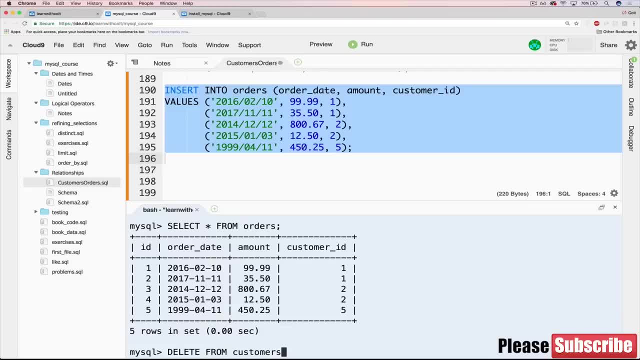 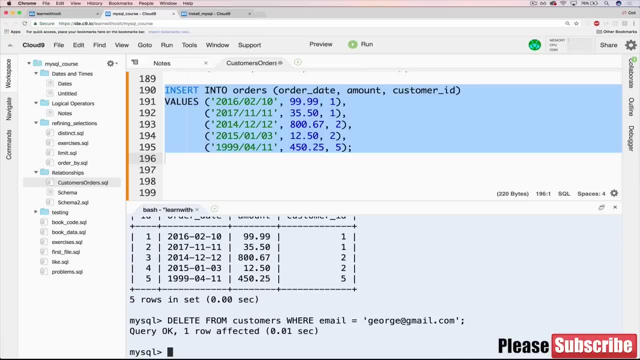 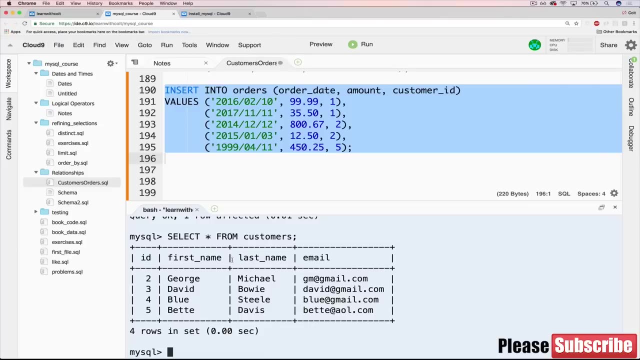 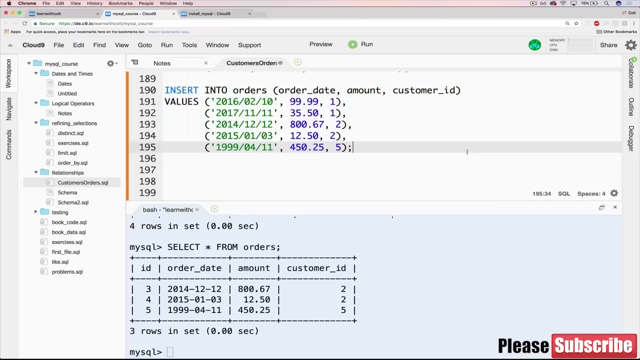 going to delete from customers where email equals George at gmailcom and we don't get that scary error. Now, if we look at all our customers, we're missing boy George, and if we look at our orders, we're only down to three. All right, now we're about to move on to our exercises, So you're going to get some practice. 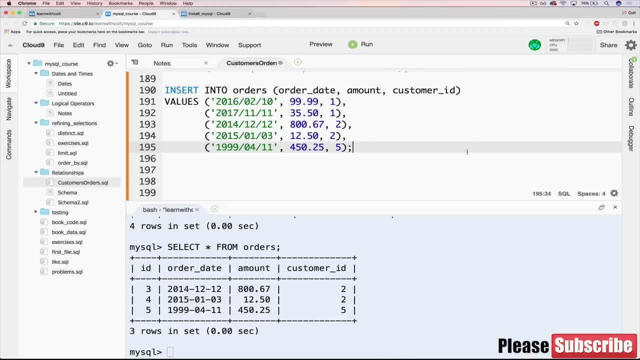 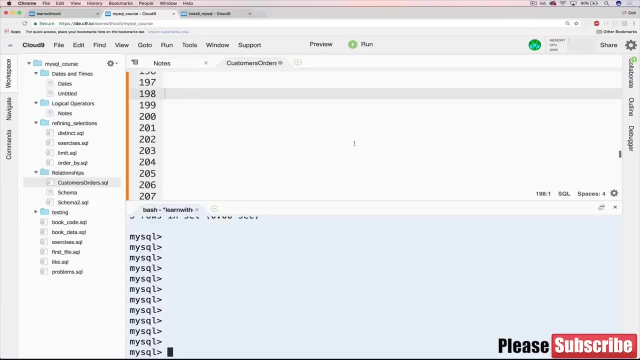 on your own. Hopefully it's a little it's. we have new data, so hopefully it's a little more interesting, rather than having to work with the same old data over and over and then we're going to keep moving on, All right, okay, I'm back with a very quick addition. This is a frequently asked 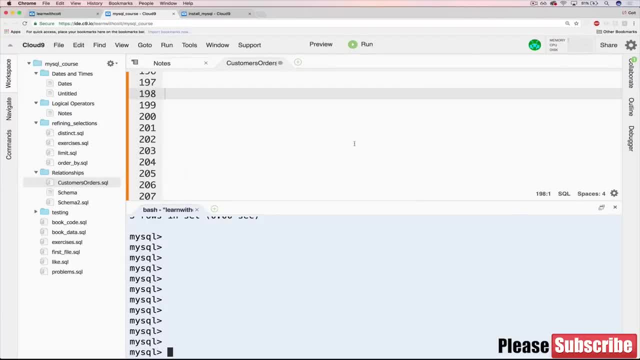 question that I get pretty often, which is: is there really a big difference between right and left joins if we just change the order of what we're joining? and the answer is no, they're actually the same. So if we do a left join- where this is customers a, and then on the right we have orders, 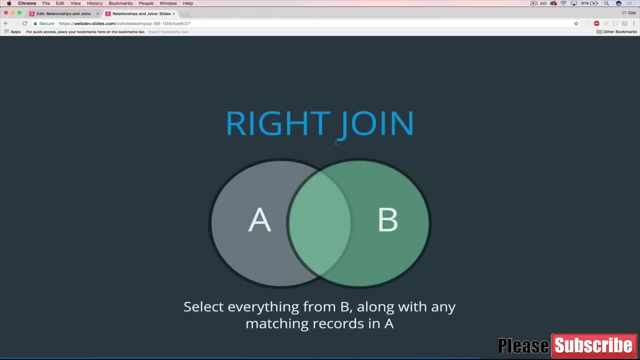 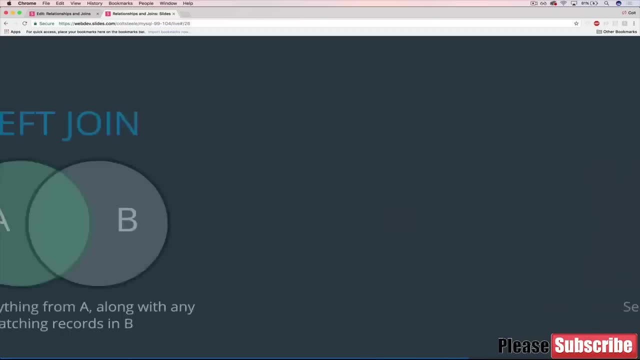 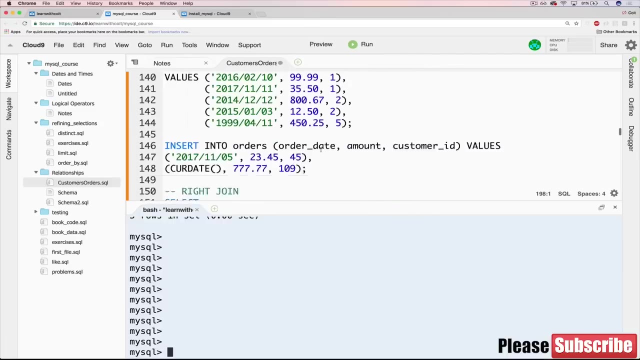 that's identical to doing a right join. if instead we put customers over here and we put orders under a, So think of it as just you know, flipping this, There's no difference. So let me show you an example: If we go, and we go grab our simple left join from way back here, this one right here. 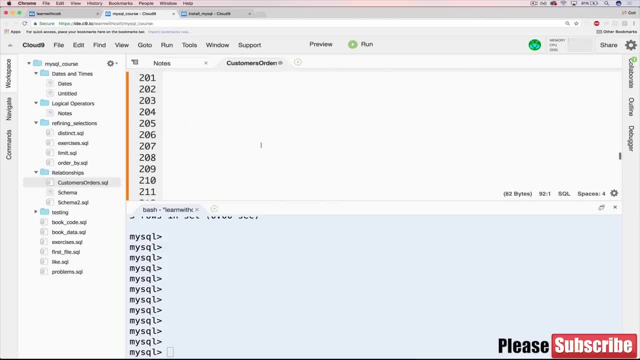 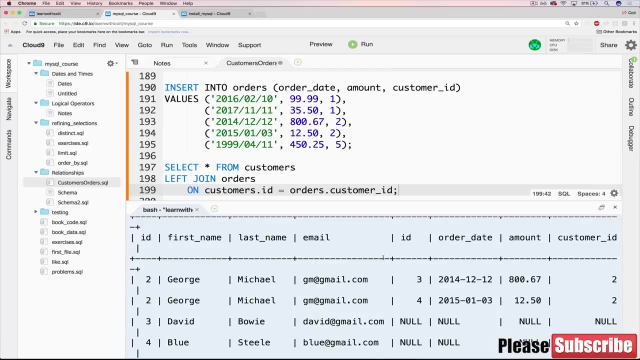 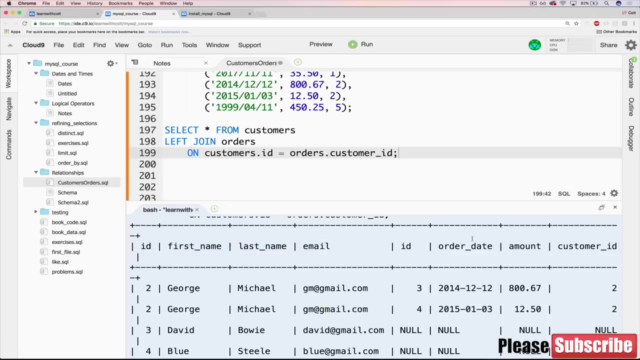 Simplest left join and I will paste it down here, just so you have it to see and let's paste it in as well. Okay, first of all, there's a lot to look at right, But what's most important is that we have, on the left, customers information first, and then on the right we have our order information, right? 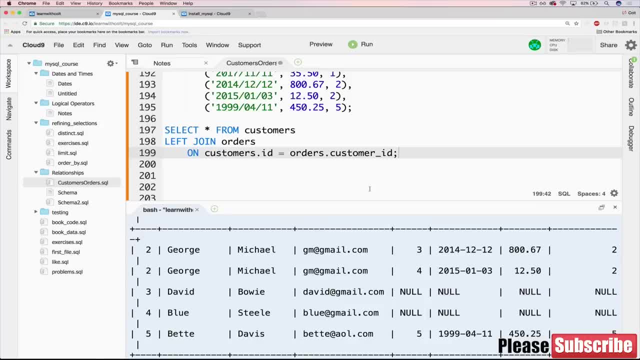 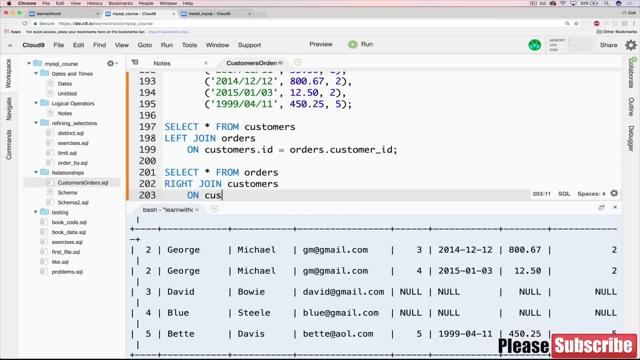 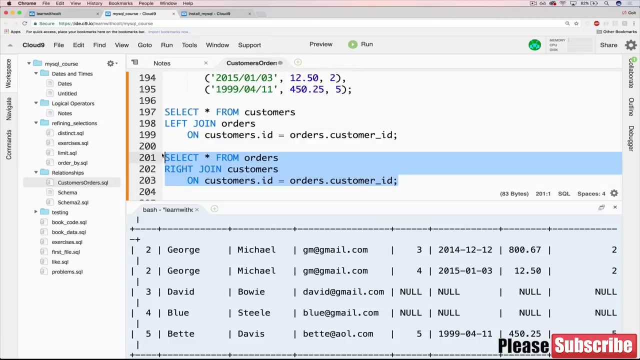 and then we have nulls where we don't have a matching order. Okay, so what happens if we try to do this? Well, we do a right join management first, but instead of doing customers first, we do orders, And we do a right join customers on. Customers to ID equals orders dot customer ID. 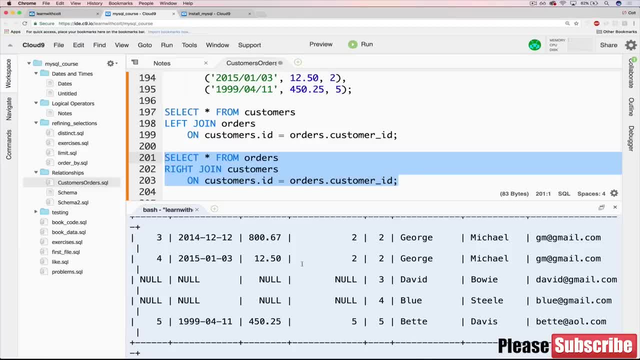 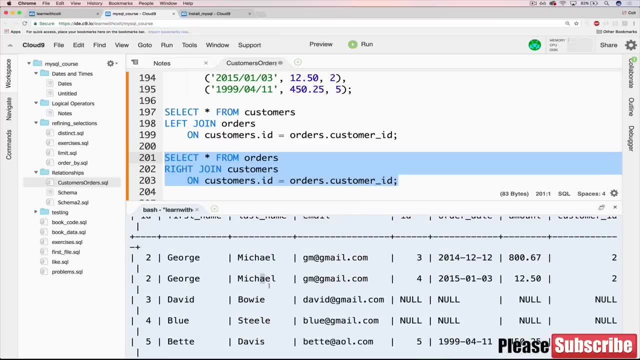 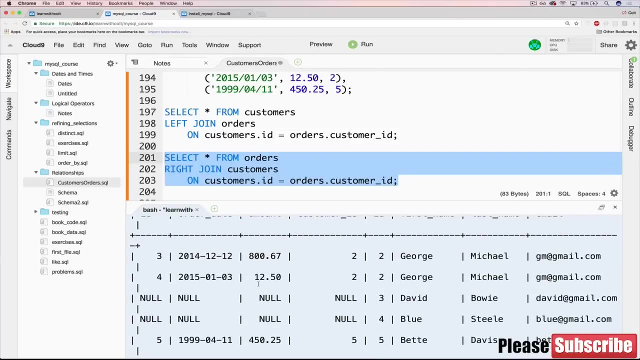 Okay, so if we do this, Look at what we get here. So we have the exact same data: one, two, three, four, five, rows 1, 2, 3, 4, 5.. But the order that the printed is different, right, so we have on the left side. now we have our orders information. 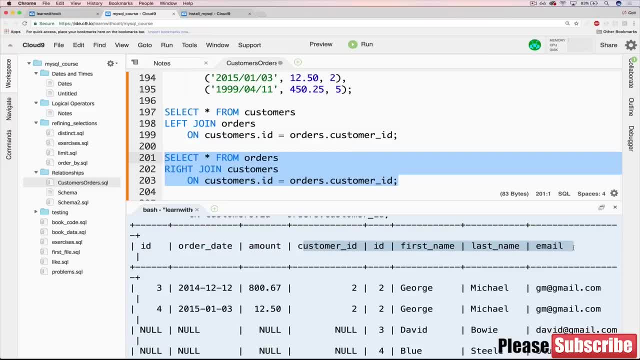 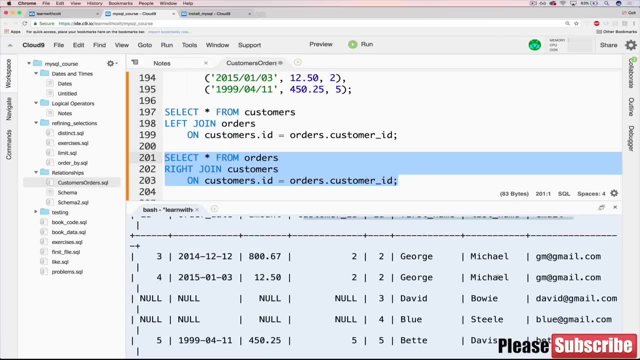 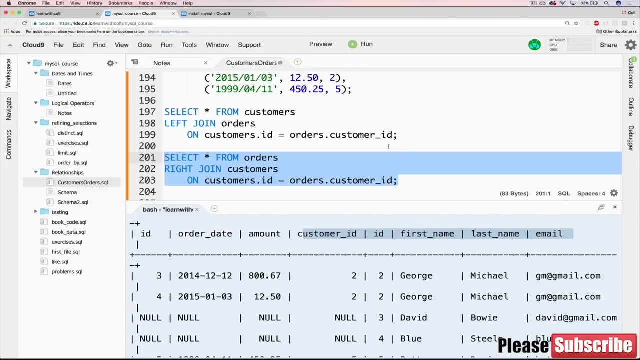 and then on the right, we have our customers information, but the actual data that's displayed is the same. yes, the order changes, but that's, you know, trivial, that doesn't matter. so in effect, these are equivalent and in fact, some, uh, like some environments that i've come across, some 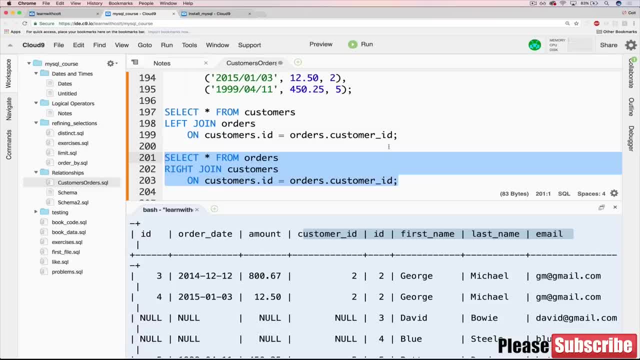 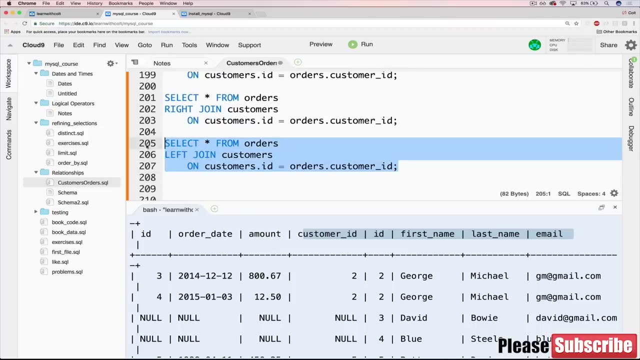 development environments won't even support a right join and they just want you to do a left join and switch the order. so to actually to sum up one more time, let's say i did the same thing here with orders and customers, but i did a left join. what would happen now? what's a left join? 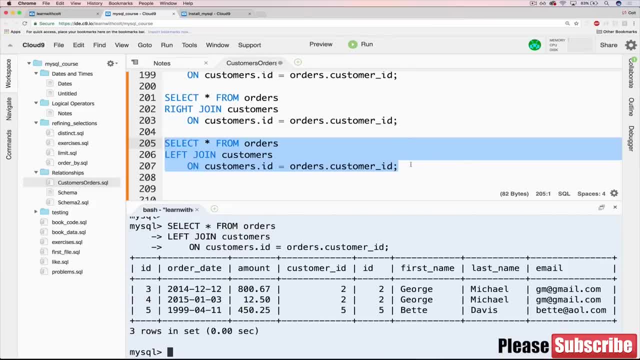 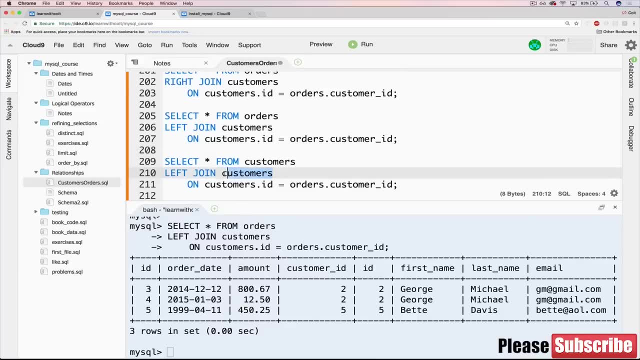 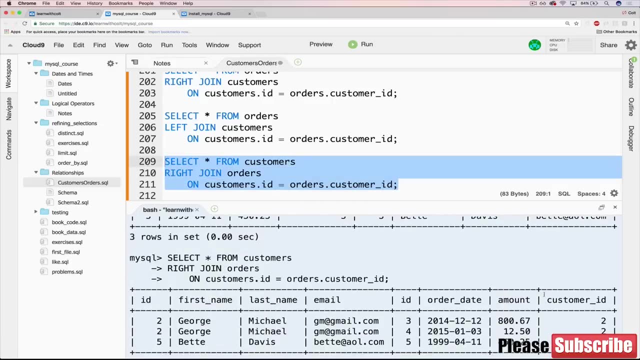 with orders first and then customers, and the answer is: it's the same as doing a right join, except if we start with customers and then orders and unfortunately we don't really have anything to see right because our data doesn't have any discrepancies on the order side. this is what the entire last 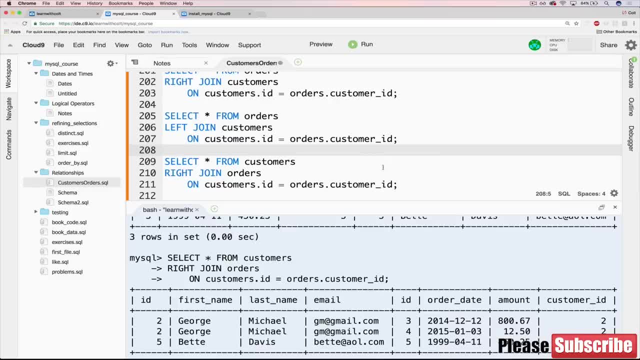 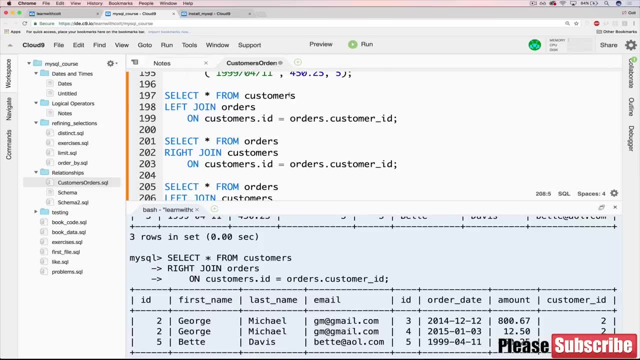 video is about, which i will not retread here, but my point is that they look the same and they look just like an inner join as well, but when we have something different, like with our left join for customers and orders, you can see that the data is actually the same. all right, so we made it. 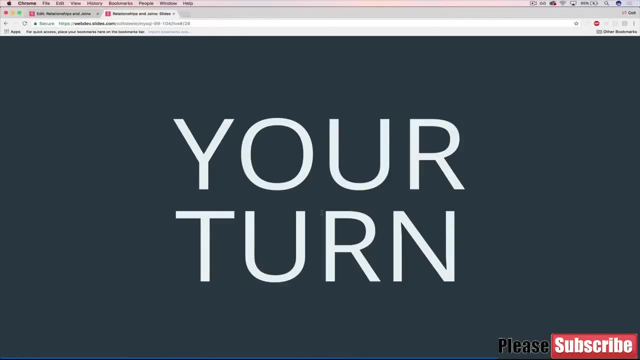 we. at least i made it through. hopefully- uh, you're still hanging in there, hopefully you're you're alive and you survived that section. i know it can be brutal. this is, for me and for most teachers the hardest thing to teach, not because it's technically that difficult, but it's a big 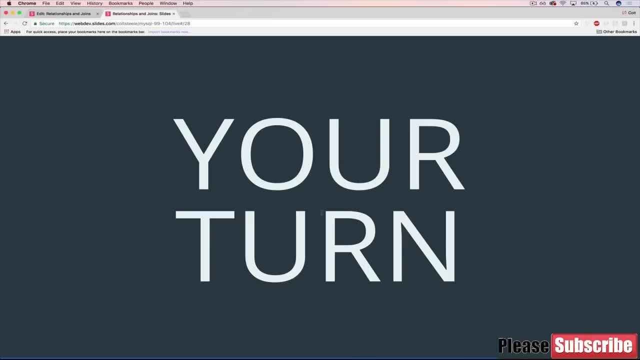 thing, we have to have multiple tables. and to have multiple tables we have to create the schema, we have to insert the data, then we have to, you know, show what the data looks like, to understand it, and, And then we can get started with the joins. and you have to manipulate the data to change. 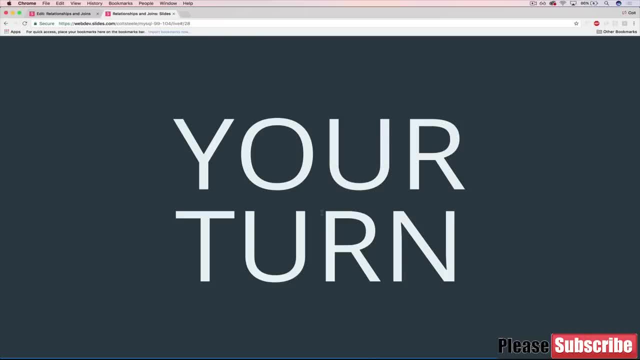 It's just a lot of work and it's tough. It's tough to keep it engaging And frankly, I don't think that that was terribly engaging. so I'm sorry. Hopefully you made it and I'm doing my best to make the rest of these a little bit more exciting. 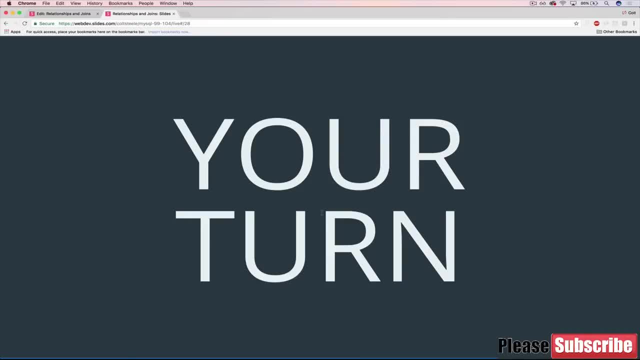 because once we have these tools in our belt, it's a lot easier to start doing case studies- which we'll be doing- or making a full application. We're getting close to end products, to actually making things rather than silly, one-off little examples. 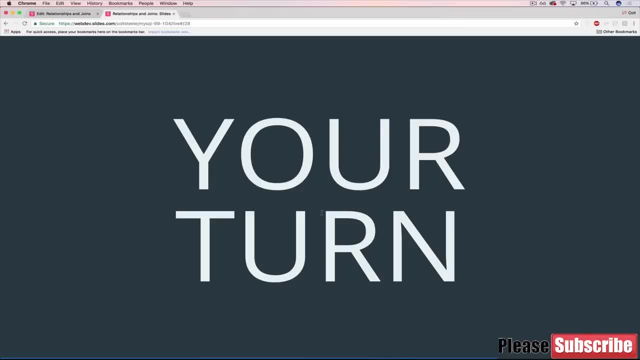 Okay, so it's a long preamble. It's now your turn And this is where you're probably- if you're confused, if you're stuck with this, join stuff. this is hopefully where you'll be able to make some big connections, to have some breakthroughs. 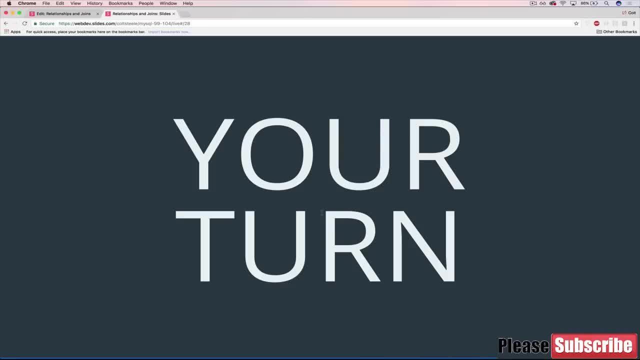 So this is a little different than exercises we've done in the past. There's only one schema, one table you'll be working with, And we're going to do that, And we're going to do that, And there's not even that many questions. 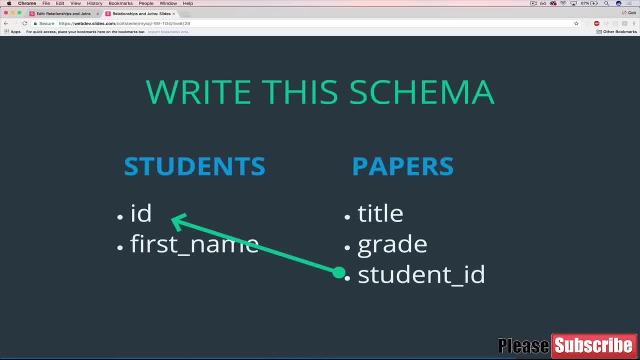 But the first thing is that we're going to be working with students and papers, So I'm a teacher. let's suppose I guess I am a teacher. but let's say I'm working in a classroom with high school students in an English class or a literature class. 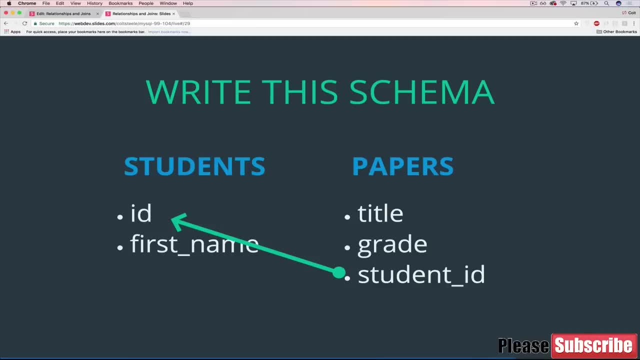 It's going to be very, very simple data. I'm telling you what I'm looking for: Students and papers, And for students, we'll only worry about an ID and their first name, So don't even care about a last name. 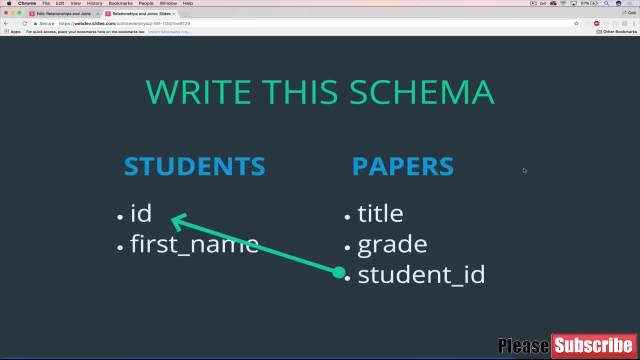 We'll just make sure first name is unique And then we're going to have papers And it's a one-to-many relationship. One student can have multiple papers, But a paper can only belong to one student, So these papers will have a title, a grade, a letter grade, like or not a letter grade? 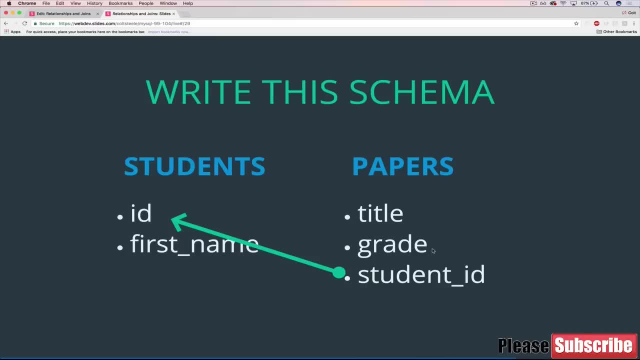 a numeric grade, excuse me, like 90 or 60, if they don't do particularly well- And then a foreign key student ID which is referencing the student ID. Okay, So that's the basic schema and I'd like for you to first go. 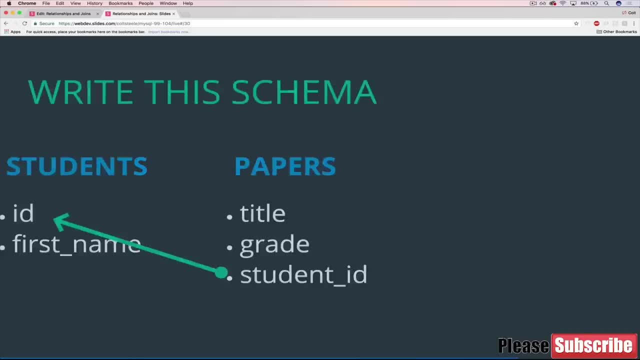 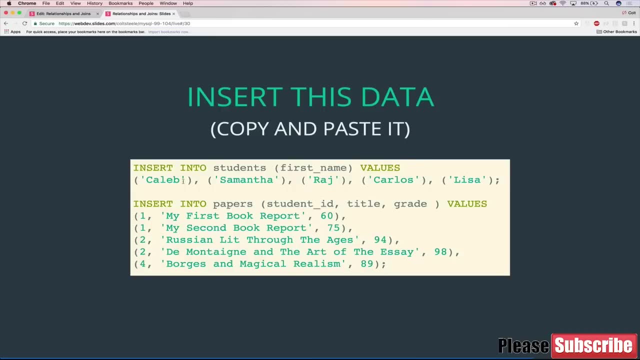 through and actually implement this. And don't worry about the data, because on the next slide I'm giving you the data. you can copy and paste it in. So this data is what we'll be working with. So we have one, two, three, four, five users. students. 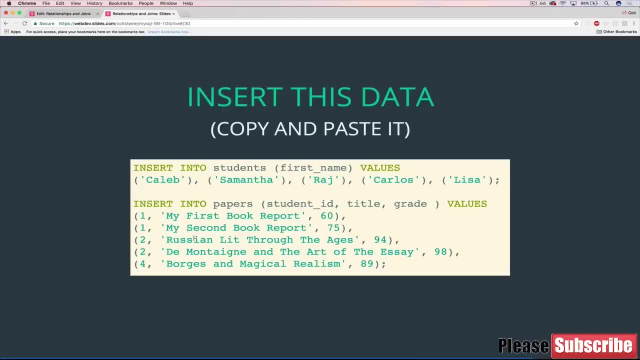 I keep doing that, And then we have six. no, I can't count five different papers, But there's a couple important things. One is that a couple of students actually have multiple papers. So, for instance, if we take Caleb, 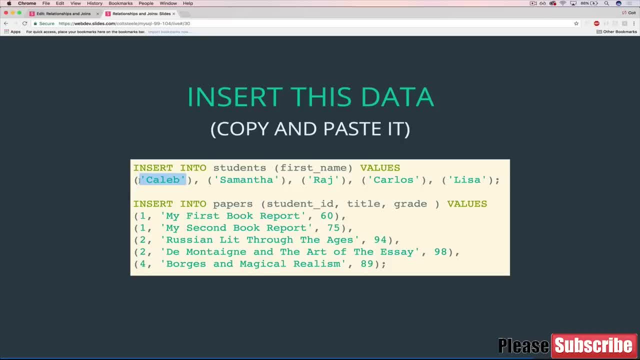 His ID is one, although you can't see that here, but he's the first one inserted, So his ID is one, and he has my first book report, which didn't get a great grade- 60%, and my second book report, which only did marginally better 75%. 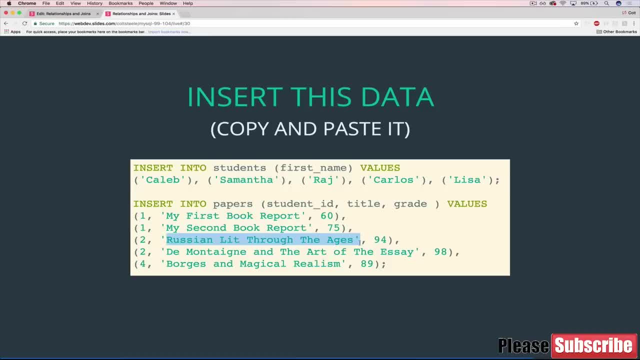 Then we have Samantha, who wrote Russian Lit Through the Ages, And we also have another paper by her, De Montaigne and the Art of the Essay, And then Raj. it looks like we don't have anything from Raj, where his ID is three. 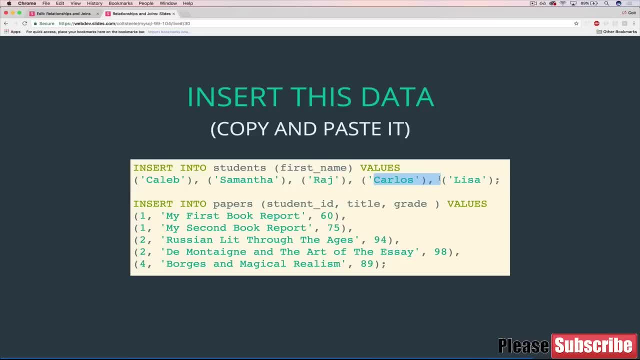 I don't know why. I don't see anyone or any paper with ID of three. Then we have Carlos, who wrote Borges and Magical Realism, And then we have Lisa, who didn't submit anything either. So let's say, and the whole point of this is that it's the end of the year and I'm trying to figure- 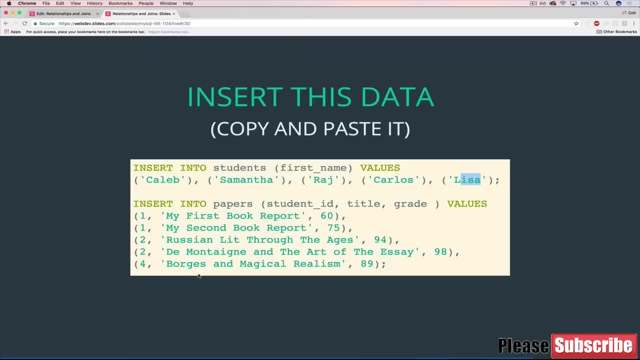 out who submitted what papers, what their average grades are. If I need to, you know, talk to somebody about they didn't turn anything in, who's going to fail, and so on. So here's the data we're working with. 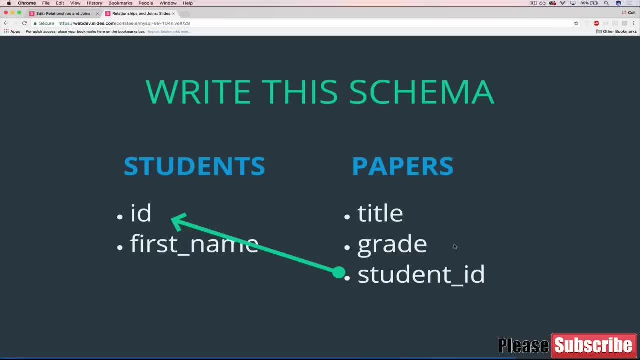 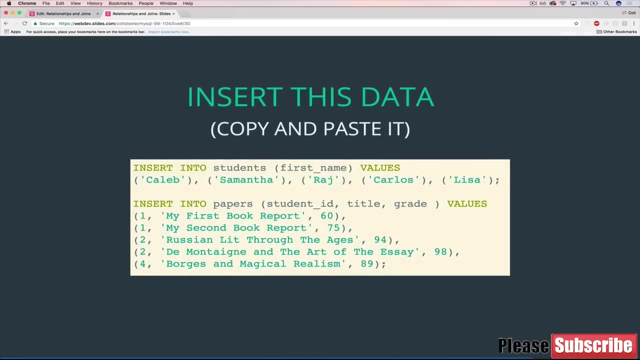 But the first thing you need to do is write the schema. So just again, to reiterate: primary key, foreign key: Varchar, varchar, integer, integer. Okay, Moving on, Once you have that done and you have your data in, you can play around with it. 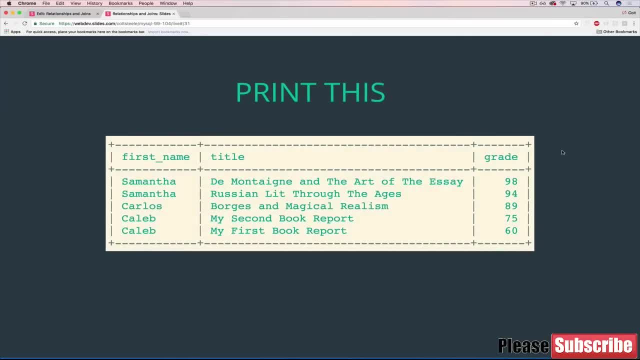 But I'd like you to print this first table. So all that we have here is first the name of a student and their corresponding paper, the title and the grade: Samantha and her two papers. Carlos and his paper. Caleb and his two papers. 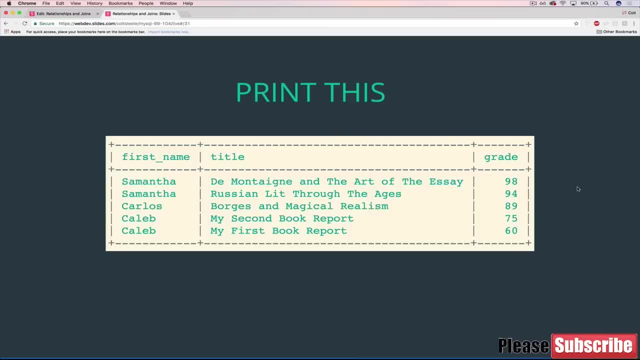 and then the corresponding grades. So this is a join. What type of join is it? And you only need these three things. So I don't want to see ID. I don't want to see student ID, just first name, title and grade. 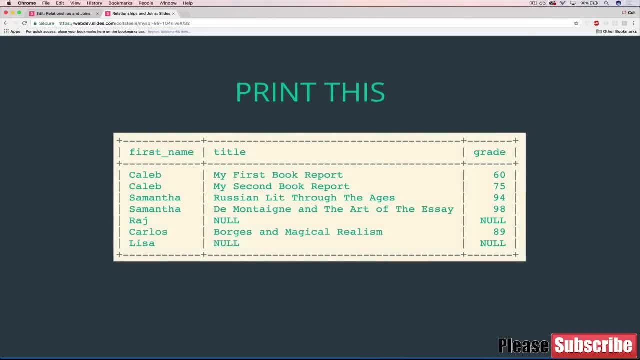 And then, once you've done that, we have another join. I'll give you a hint: Everything in this section, in this exercise, involves a join. This one is different Because we have the same basic stuff: Caleb and his two book reports. 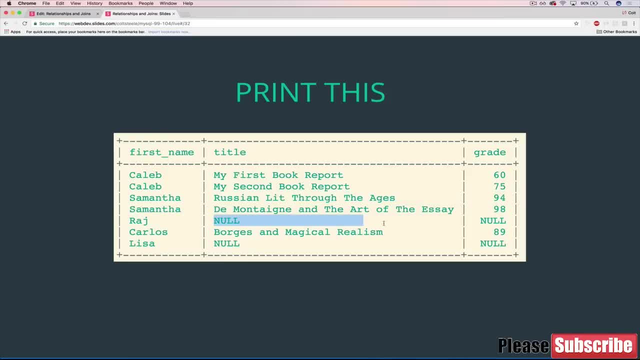 Samantha, her two papers: Raj, though, null title, null grade. Raj didn't have a paper. Carlos Borges and magical realism. and then Lisa, null, null, Lisa doesn't have a paper either, So print this out. 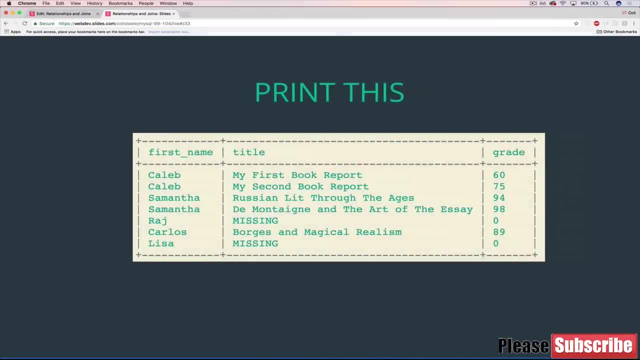 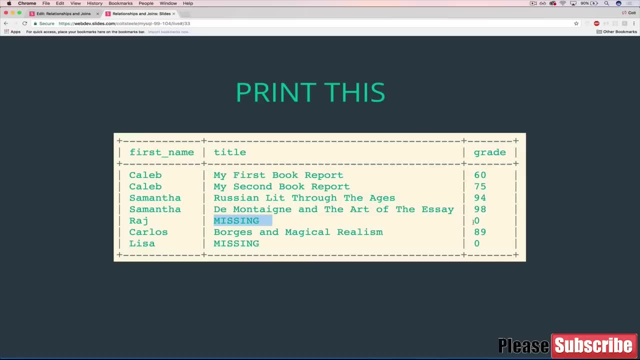 It's a different join Then, once you've done that, move on. Similar. but notice, instead of having null and null when a student didn't turn any papers in, we now have missing and zero for their grade. Missing for title, zero for their grade. 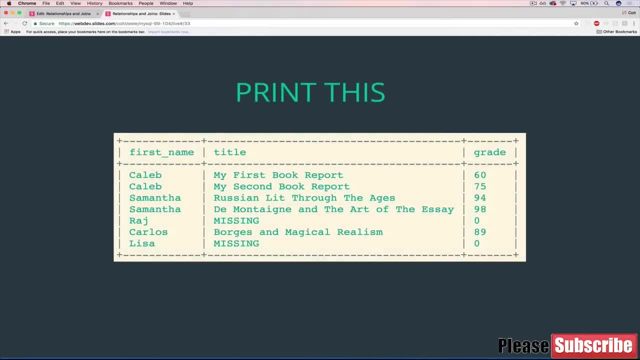 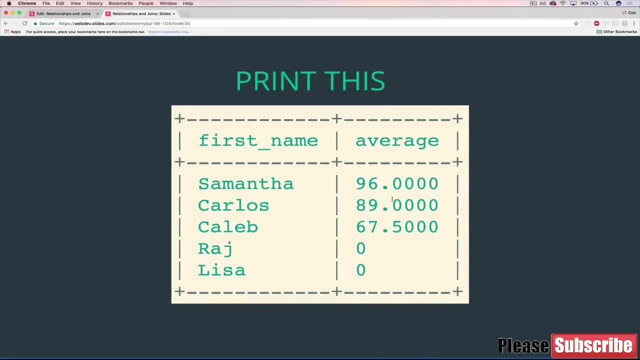 So it's the same thing here. we're just subbing in. Okay, Then we get to this. This is going to be an average grade next to every student. So we have Samantha, and the average of her two papers is 96.. 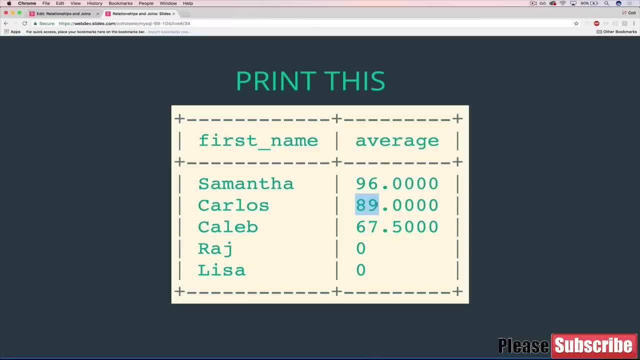 Carlos, the average of his one paper is 89.. Caleb's average for two papers 67.5.. Raj has an average of zero because he didn't turn a paper in, And Lisa has an average of zero as well. So I won't give away too much about this. 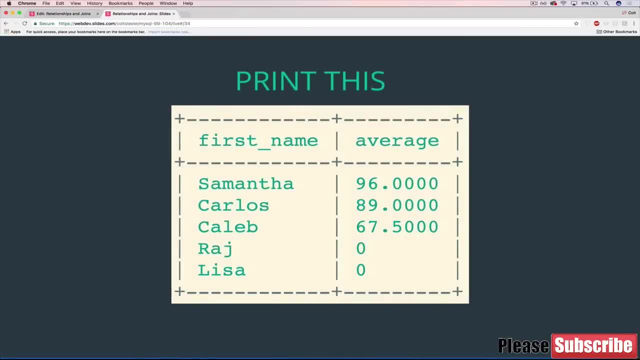 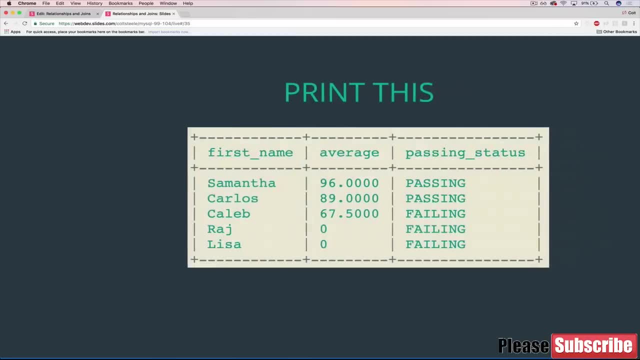 but you can use the same join you used here. You just then need to condense it. We need less information, You'll need to. well, I'll leave it at that And then finally print this, An extension of what this one was, except there's a new column. 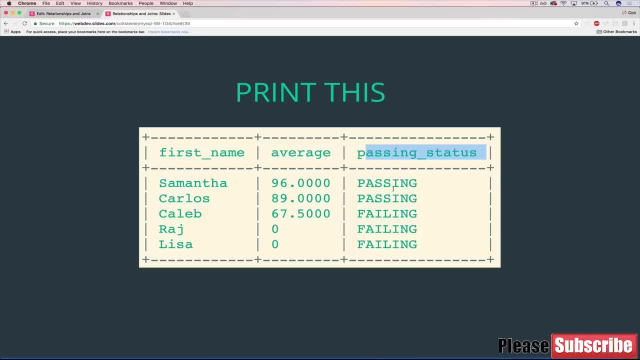 which is passing steps And passing status just says if the student is passing our class or not And the threshold. I should have written this out. The threshold is if they get a 75 average in the class or higher. So Samantha passes. 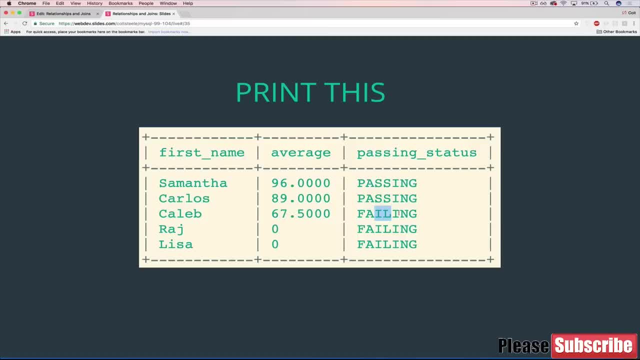 Carlos passes. Caleb, unfortunately, is below 75. So he fails, as do Raj and Lisa. All right, So there's a bunch of joins you need to write. First things first, though, get the data in there, Create the schema, get the data in, play around with it. 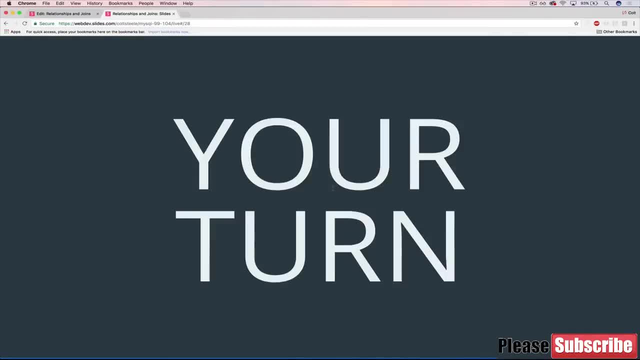 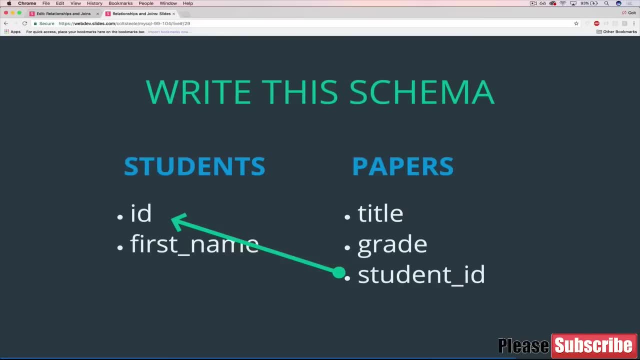 and then attempt zero. So I'm going to create these how many five joins, And I'm back here with a solution or multiple solutions to go over these join problems. So again, this was a one-to-many relationship: students and papers. 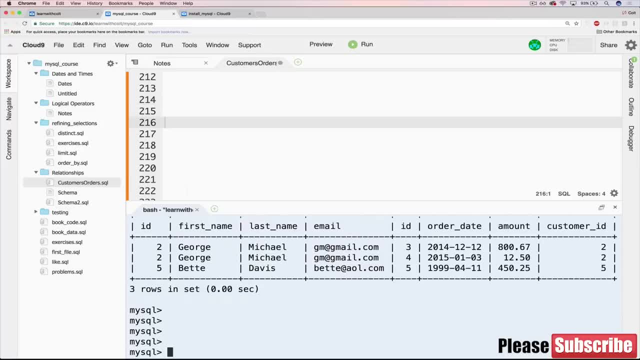 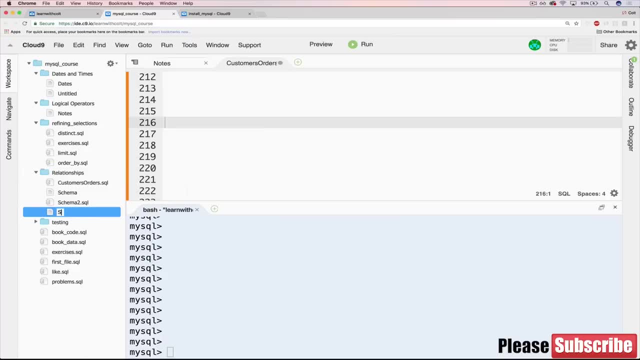 And the first thing we're going to do is go over to Cloud9.. And I'm just going to work in the same database, but I'm going to make a new file, just because it's getting crazy, And I'll call this one: studentspaperssql. 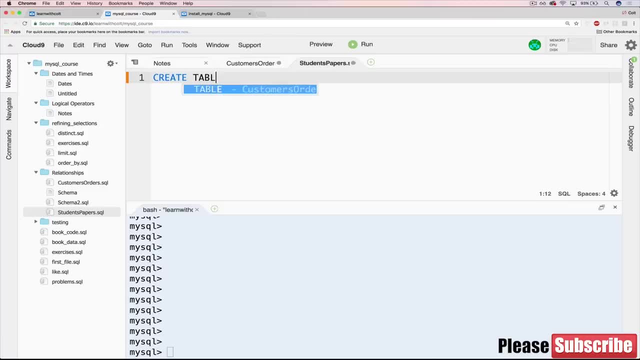 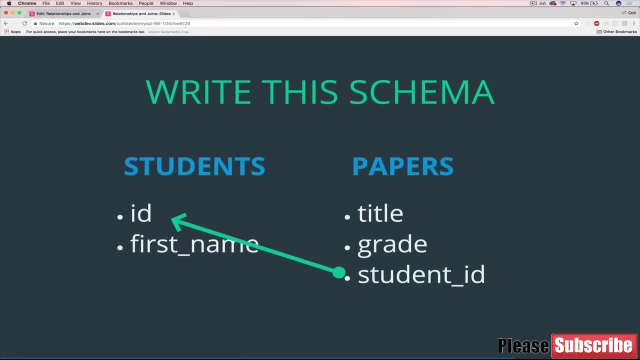 Okay, So we know we need to create two tables. Create table students- I'm just going to leave it empty for now- And then create table papers. Also leave it empty. Great. So next, what do we put in them? So we'll start with students. 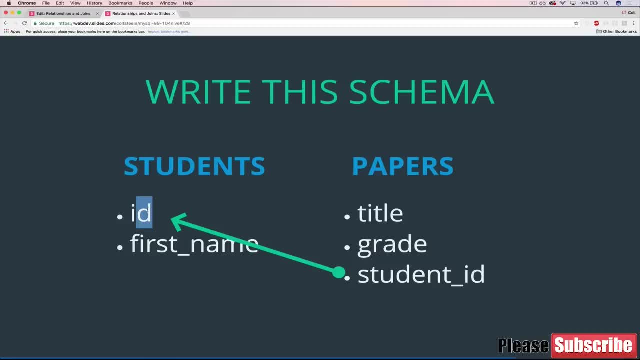 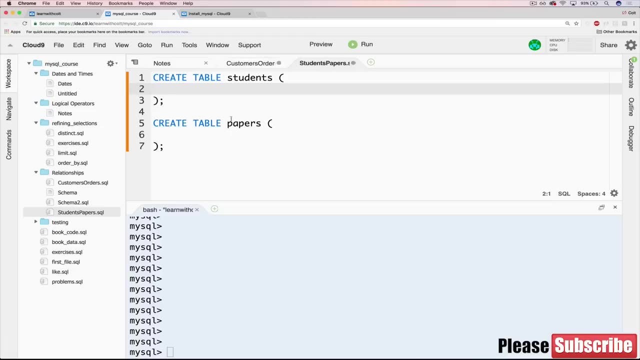 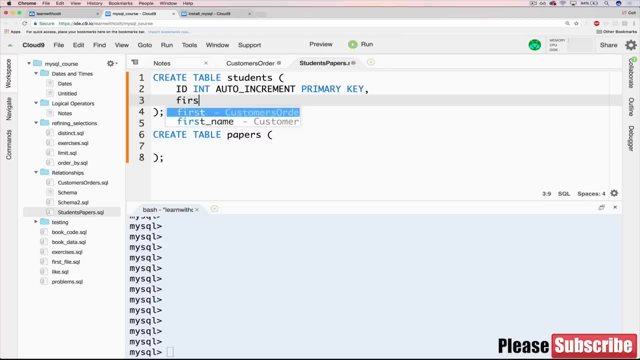 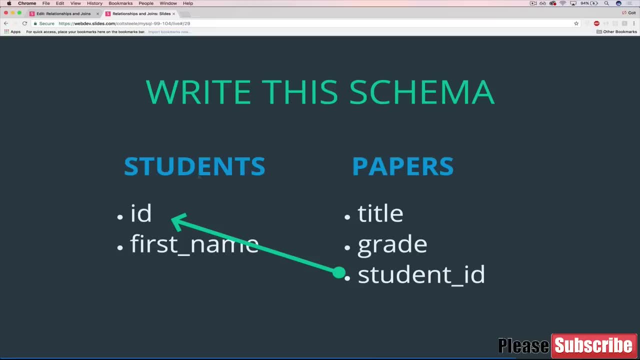 Primary key. And then we have first name, which is just varchar, and we'll do 100. It's a good, even nice, number. So that's it for students. But then we have papers. So papers has a title, grade and student ID. 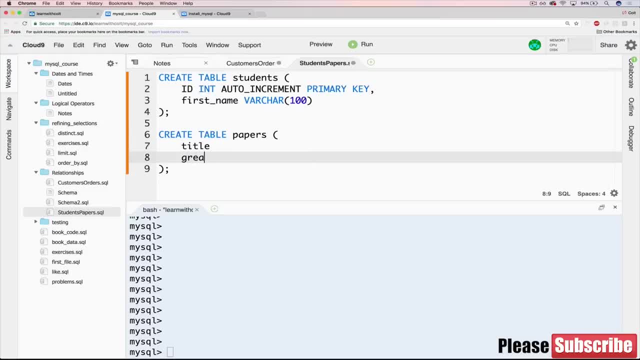 Let's start with just title, grade, student underscore ID: Perfect, And I'm noticing. you know I capitalized this. It doesn't really matter, But it's going to be annoying to remember that, So I'm just going to put it back as lowercase ID. 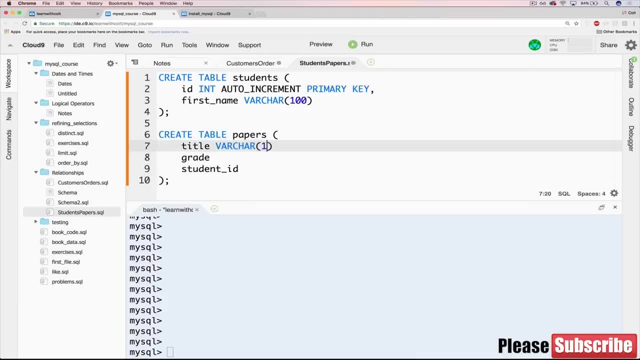 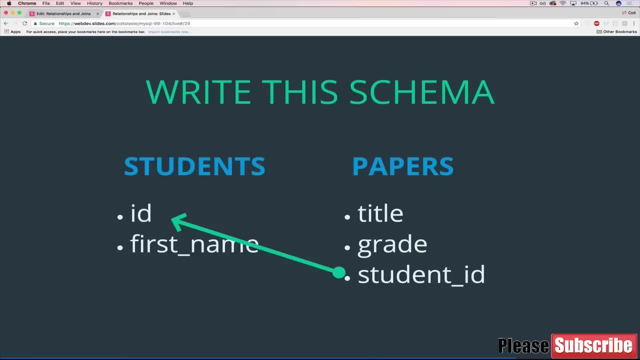 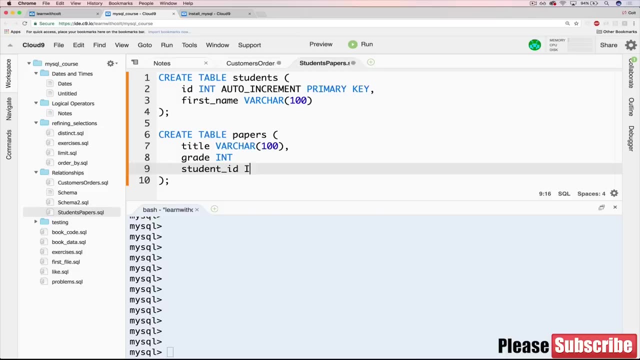 So we've got title, grade and student ID. Title is a varchar. We'll also do 100.. Grade is an int. And then we have student ID And student ID is a foreign key referencing students dot ID. So it's just an integer. 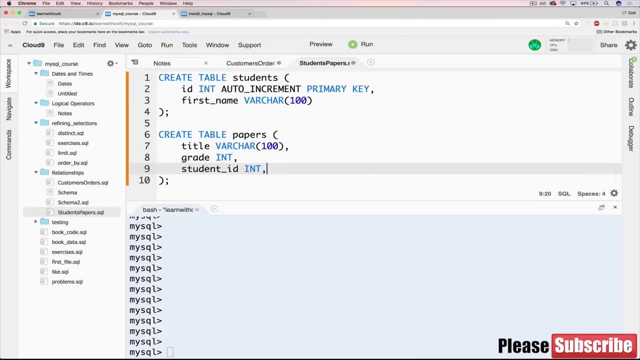 And this sometimes trips people up, that we just write student ID as an int and then the next line is foreign key. The field that is foreign key is student ID. this right here And we need to say what it references. So it's referencing students. table the ID field. 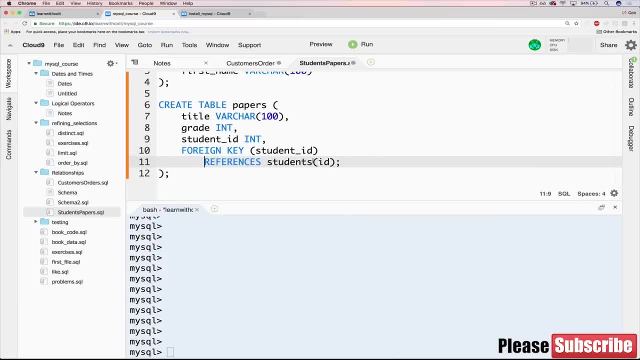 Okay, And we could also indent it like this, because this has to do with this, And then, if we wanted, to, which you did not need to do, but this is where we could add on delete cascade, Which you may. we saw in the last video or two videos ago. it's not necessary here. 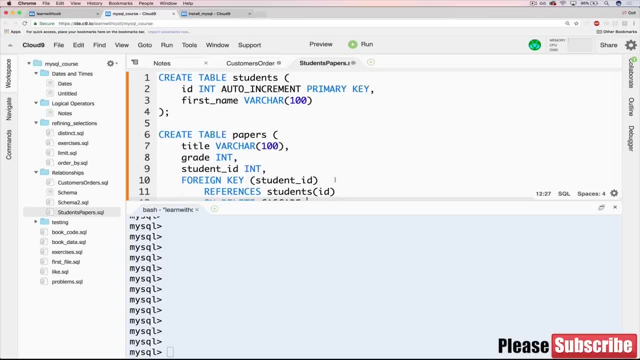 We're not deleting anything, But you could put that there, Okay, So the next step is now just to create them. So, before I go too far, I did catch this. I have an extra semicolon there. Get rid of that. 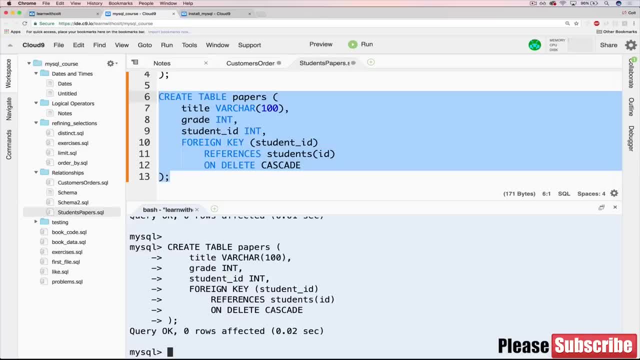 But we'll create our students table And we'll create our papers table. Everything looks good And if we do show table, Okay, And then we're going to create our students table And we'll create our papers table And then we're going to create our papers table. 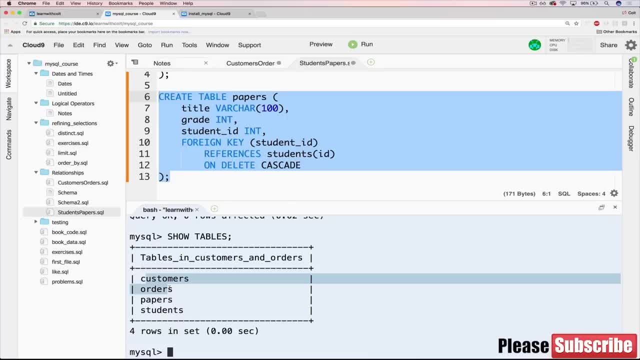 And then we'll create our papers table, And then we'll create our papers table, And then we'll create our papers table. I'm still working in our same database. So I have customers and orders- That's fine, But I have papers and students. 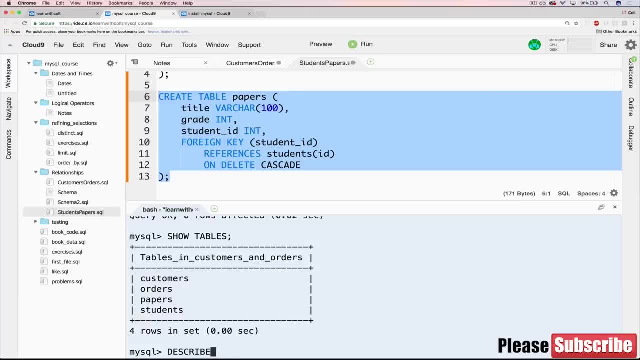 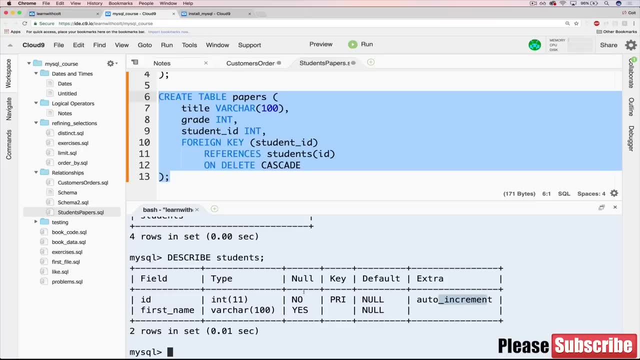 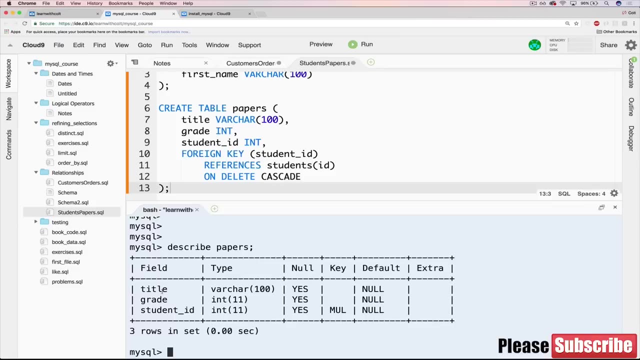 Okay, And we haven't done this in a while. How about we describe students? Cool, So we now have auto increment in there, Primary key, And that's for students. And what about papers? If we do describe papers? Well, you can see we have title and grade and then student ID. 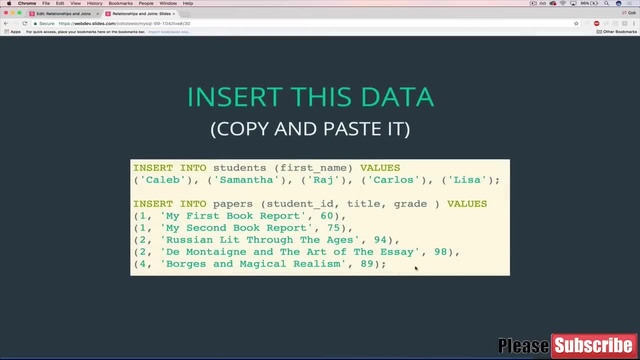 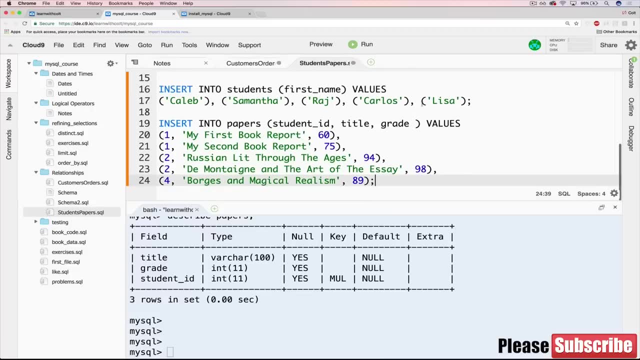 Okay, So next up is to get To get our data in there, And I said that you definitely didn't have to do this yourself, So I'm just going to put it in this file. so you have a solution file, But it would be annoying to type this. 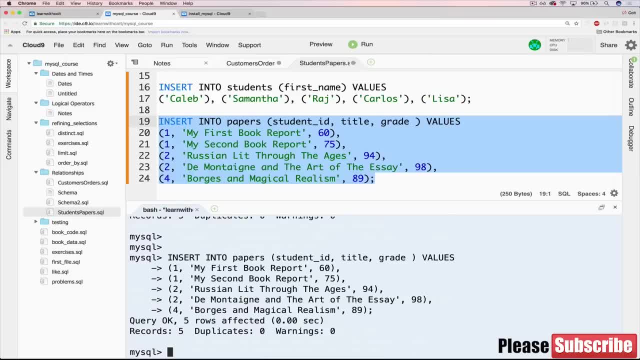 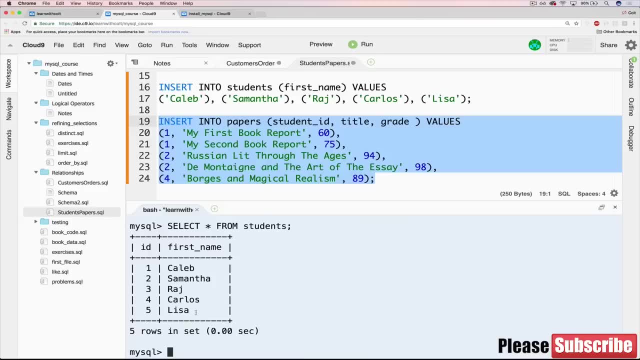 I totally. I mean, I had to type it, I totally get it, So paste that in Perfect. So now we can do a select star from students And we should see our five students And do a select star from papers. 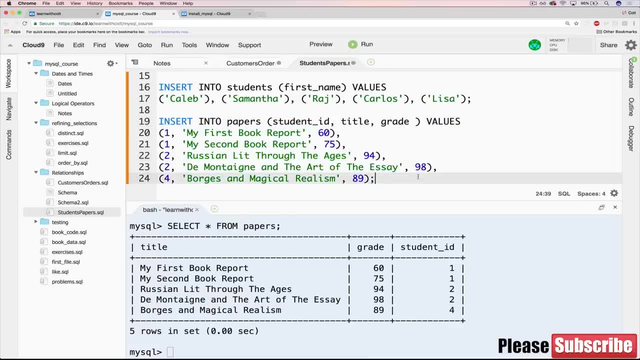 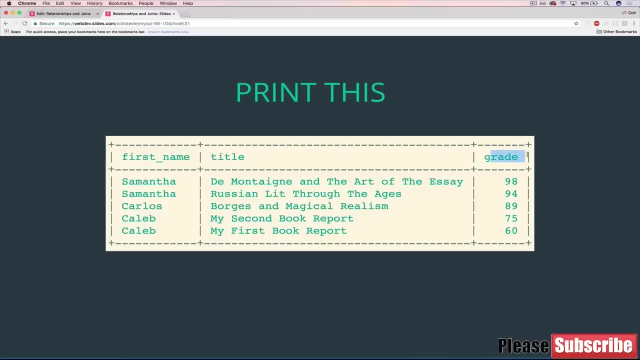 And we see our five students And we should see our five students, And we should see our five students And we should see our five papers with student IDs- Great. So the first thing to do was to print this join table Where we have first name, title and grade. 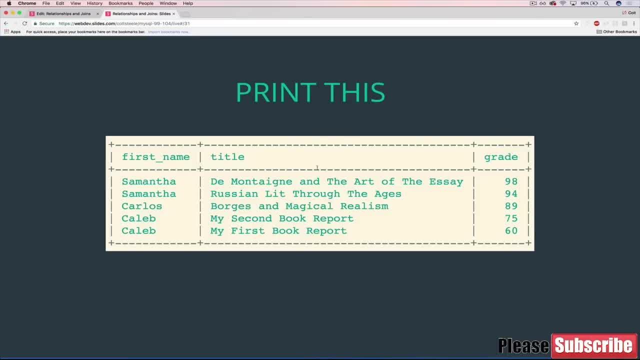 Nothing else: First name, title and grade, Where. and what's our join condition here? Well, basically, where the studentid is equal to the student ID in the paper, And this we could accomplish through an inner join. That would be the easiest way. 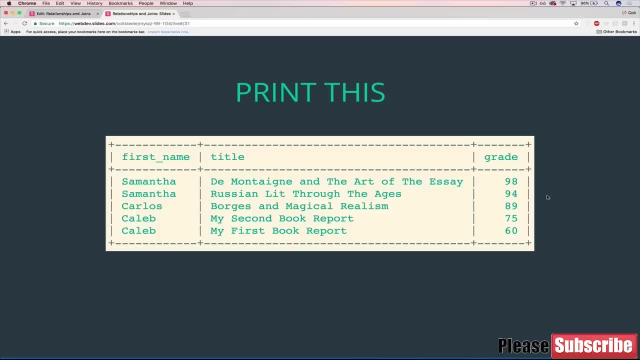 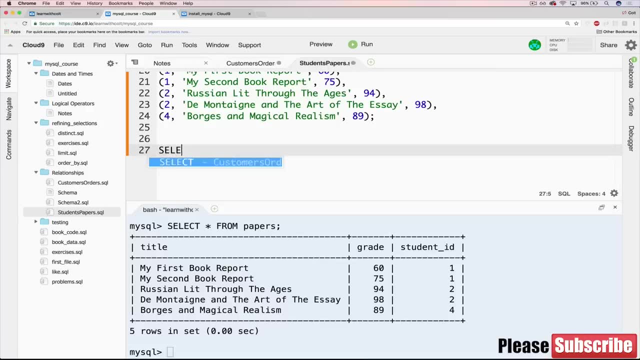 We could also do it with the right join if you wanted to, Which we'll take a look at, But an inner join is the simplest way And I'm going to do an explicit inner join. So that means select, And let's start with star from, and let me put a number here. exercise one: 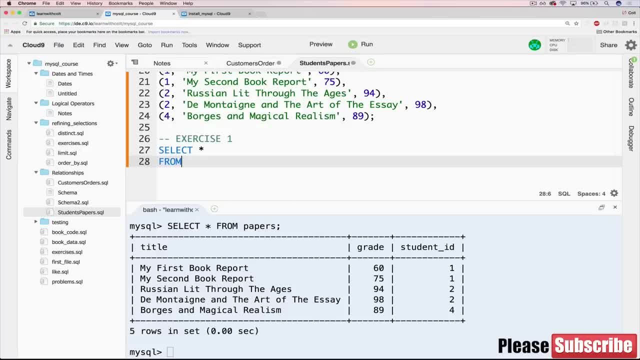 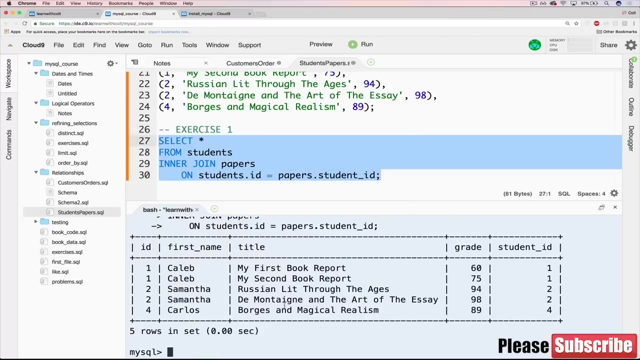 Select star from. I'll do it on a different line from students. join papers on studentsidinfo Equals papersstudentid And let's be explicit with inner join, Just like that. So if we take a look, You see we have the right data right. 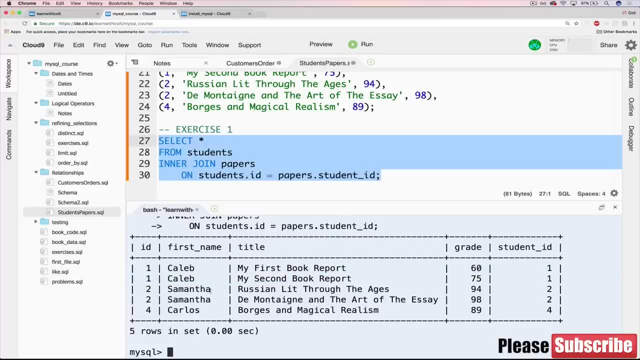 We have Caleb and his two books, Samantha, or two reports, Samantha, her two essays, Carlos and his one essay, And we have the grades. Now we don't want ID and student ID, So we just need to get rid of that. 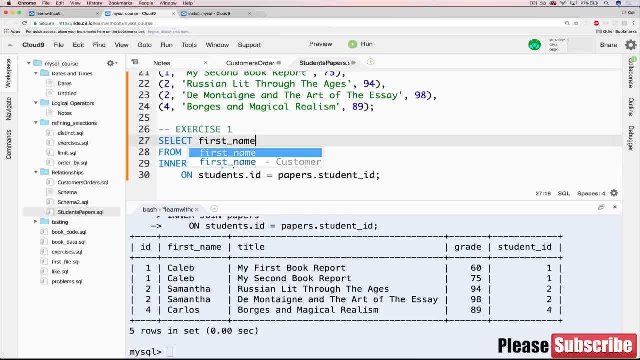 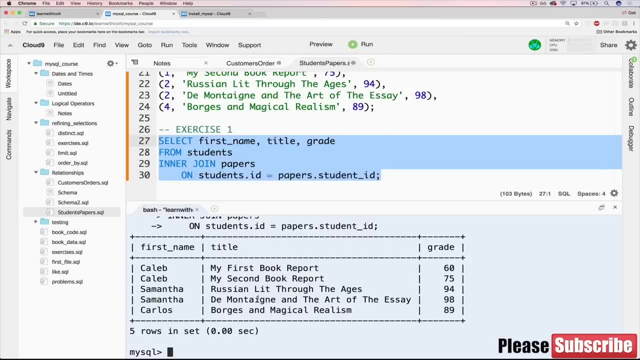 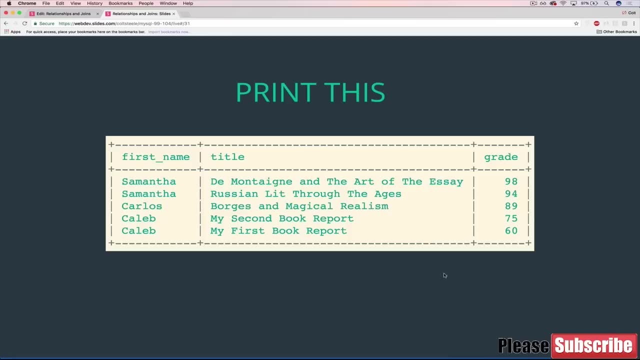 And the simplest way is just to let's explicitly say what we want. so, grade title and grade. okay, now we do it and we're good to go. there's one thing this is my fault for not mentioning in the instructions. I did order this. 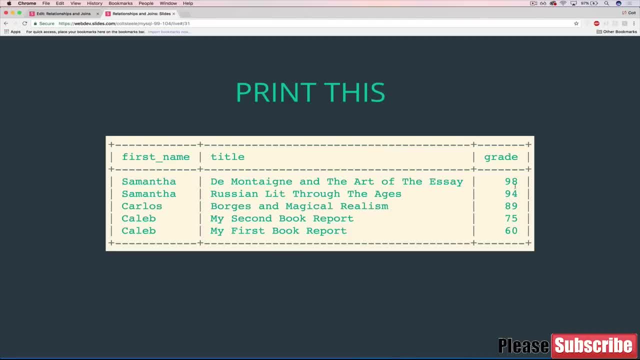 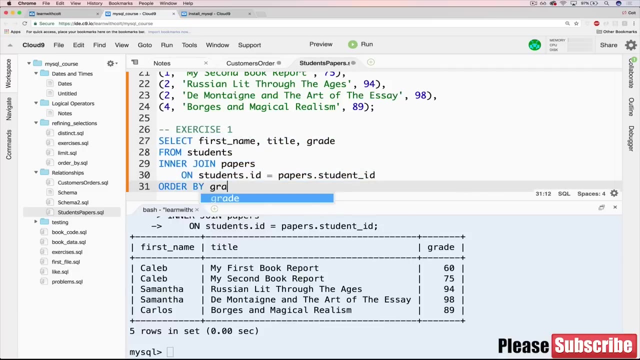 and totally fine if you didn't do it. if you did catch it, congratulations on looking at that. I didn't. I forgot I did this late last night when I created these slides. I'm recording it the next morning. so this was ordered by grade. so that's simple too. just going to be order by grade. 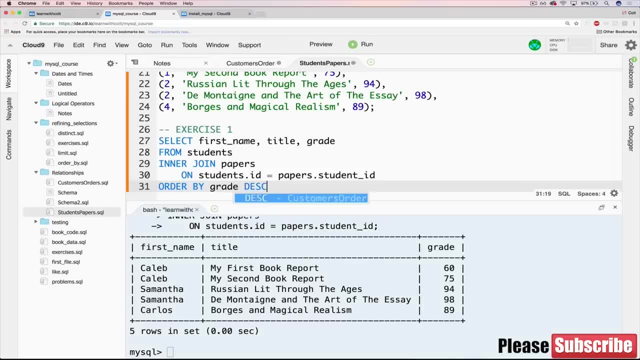 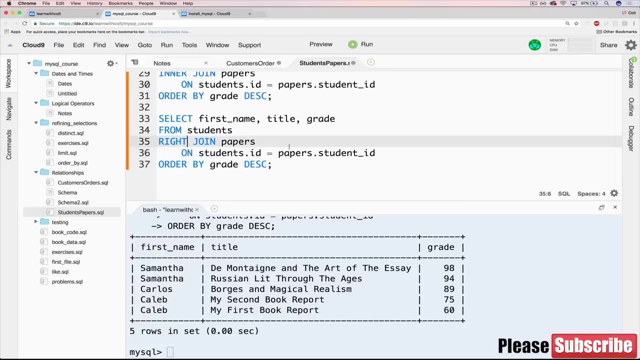 and what order is it? well, it's descending. now we do it. now we have the correct answer. the other one is correct too, I promise. the only thing that I'll address here is that I mentioned that you could also do a right join, and why is that? well, let's just verify. see if I'm crazy. 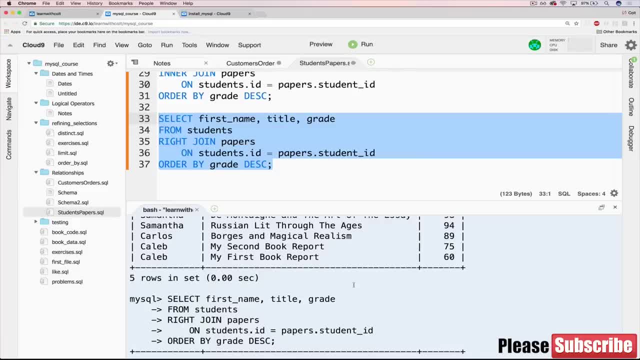 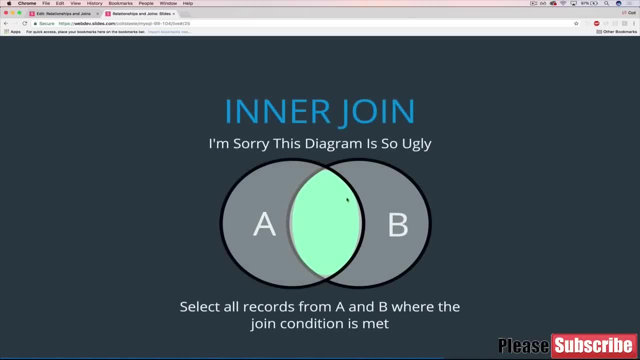 nope, still works. good to know, I'm just kidding. but the reason that it works is because if we go back to our slides way back, when we do an inner join here between students and papers, all of our papers have a student they belong to. so basically, this section is the same. 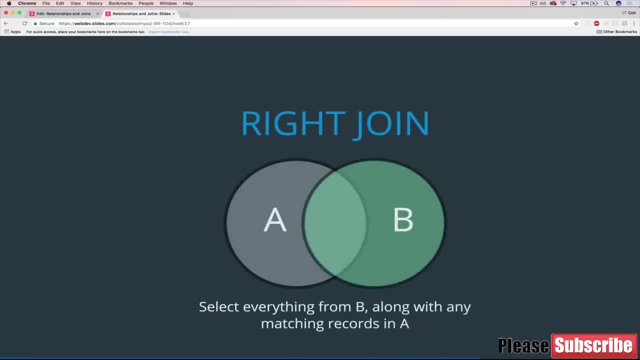 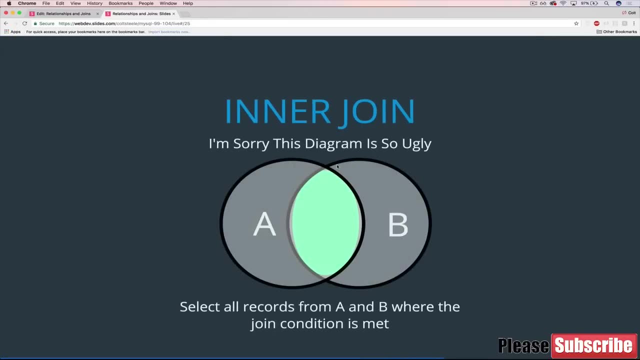 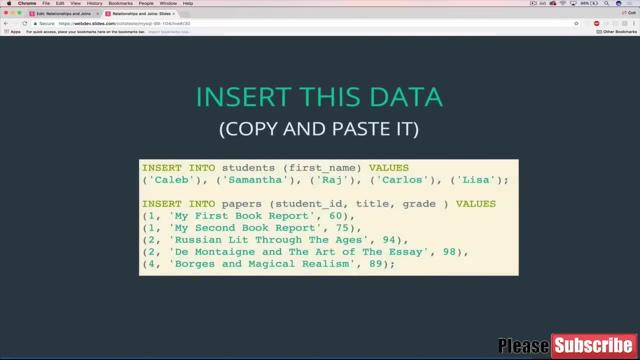 as this entire section here. the same as this. if we pretend that left join doesn't exist, ignore that slide. this intersection is the same as this because every paper has a student ID in it. so you could also do a right join- nothing wrong with that- but I think the inner join is easiest. 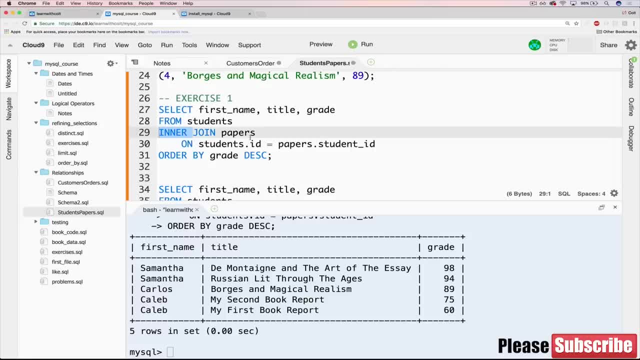 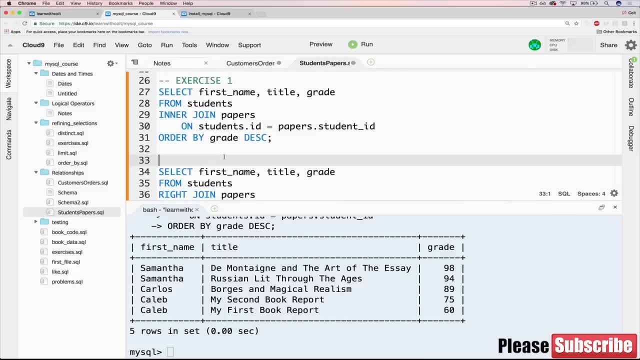 although it's easiest because it's just- this is how I think about joins most of the time- but it's not any easier because it's just a single line or a single word that we're changing okay, so I'll just write alt: solution okay. 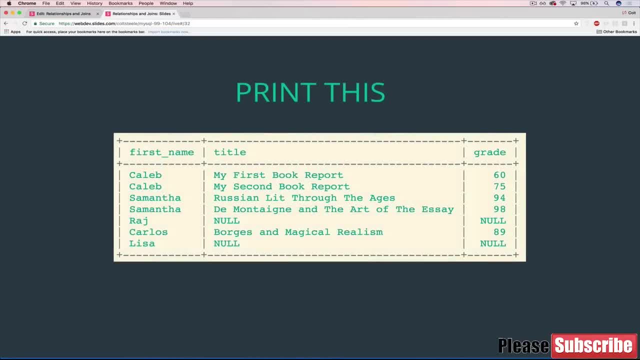 moving on, print this. so very similar right, Caleb, Samantha, their respective books, but then we have Raj and Lisa, who didn't write any reports or any papers and we have null in place. so this is a left join and the way that we're going to do that. 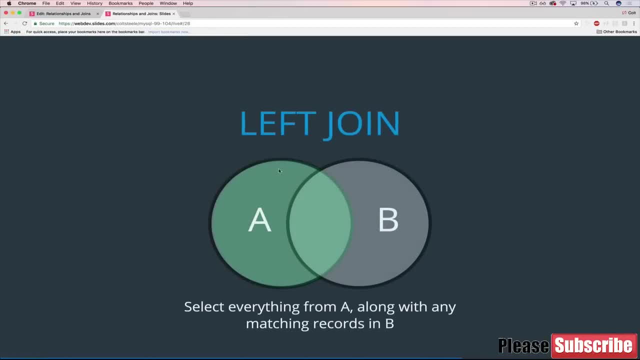 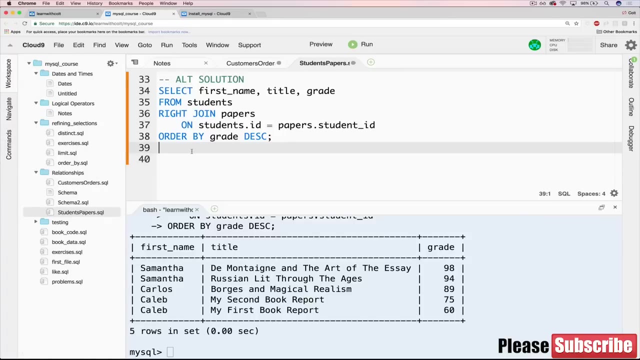 if we go back to our slides again, we're going to grab everything from students and then any associated papers, but some of them don't have papers, and those will then be filled in with null. so let's do this now call this. let's call this problem two. 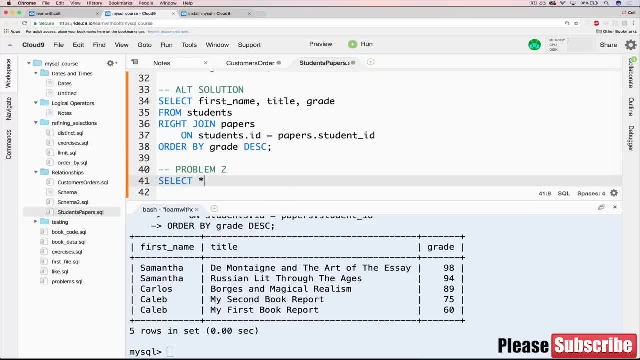 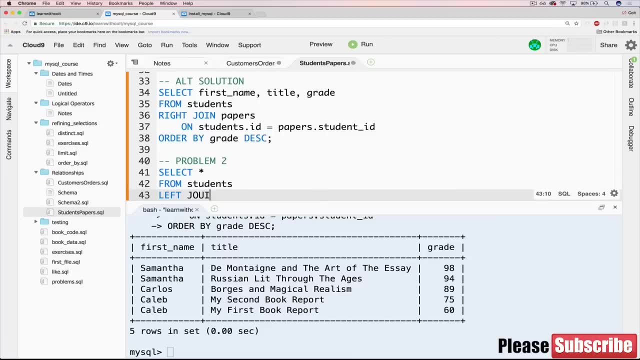 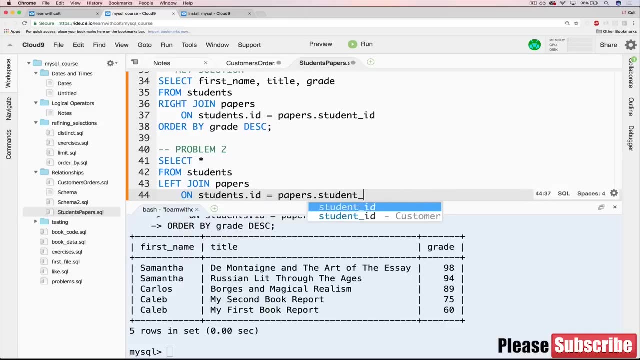 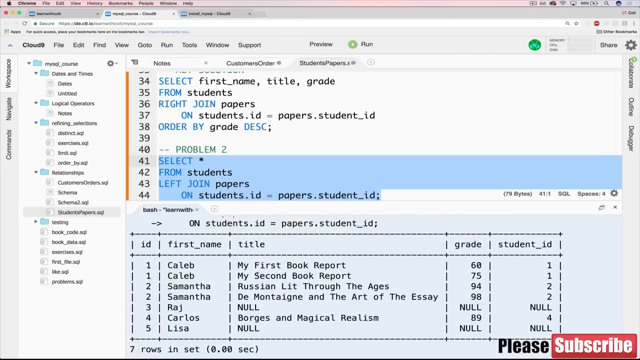 and we'll start with select star again and then we'll alter that from students and then we need to do a left join papers on studentsid equals papersstudentid and we'll leave it at that to start and you can see it's working. we've got Caleb and his stuff, Samantha, her essays, her papers. 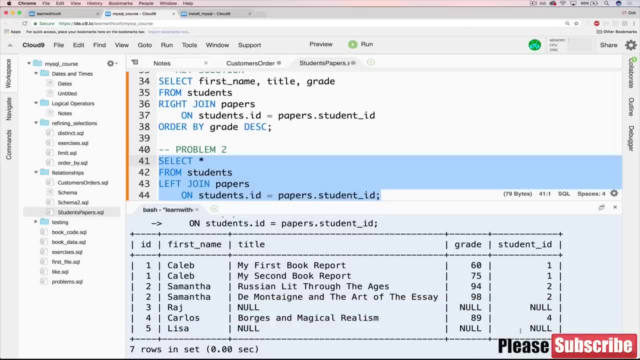 Raj, null, null, null. Lisa, null, null, null. so we're getting every single student- Caleb, Samantha, Raj, Carlos, Lisa- and if they have a matching join condition in the papers table, then we also get their paper data. 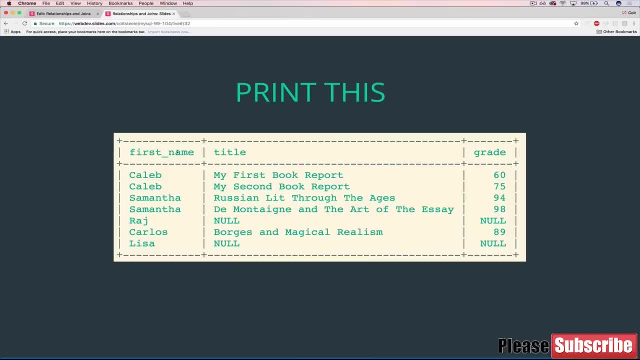 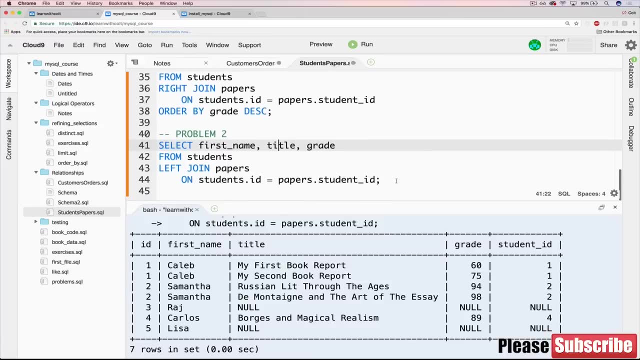 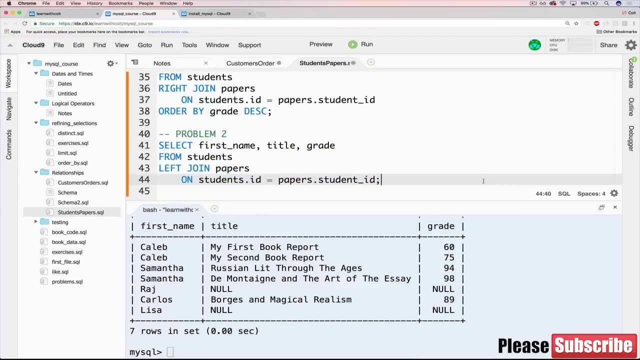 but if they don't, we have null. the only thing left is to whittle it down to first name, title and grade, just like that. let's verify, okay, and is there any sorting here? No, then we're done. okay, so problem three. 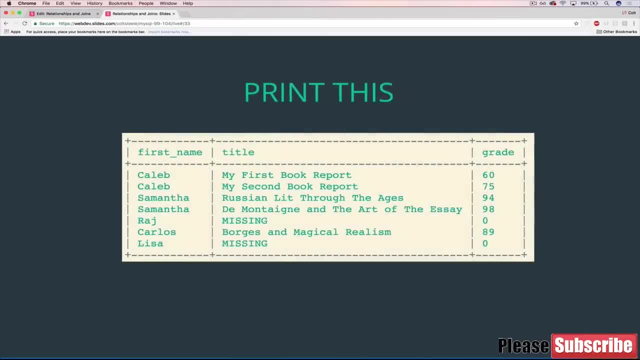 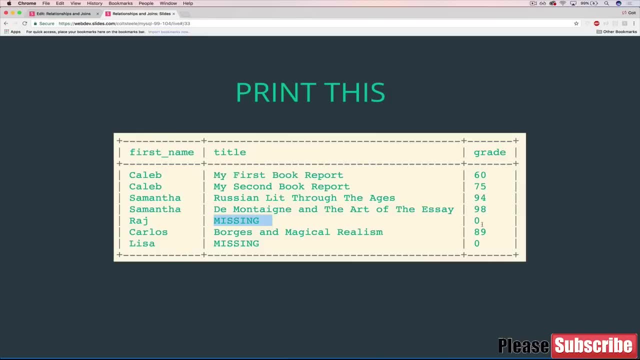 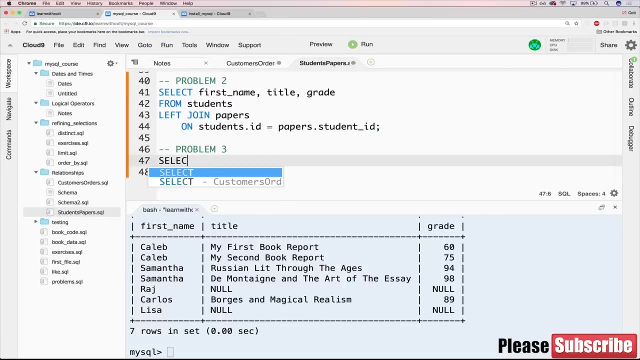 okay, it's very similar, but we're going to then substitute in for null. under title we want it to say missing and under grade we want it to say zero, so we can actually just use the same thing. so it's going to be select. 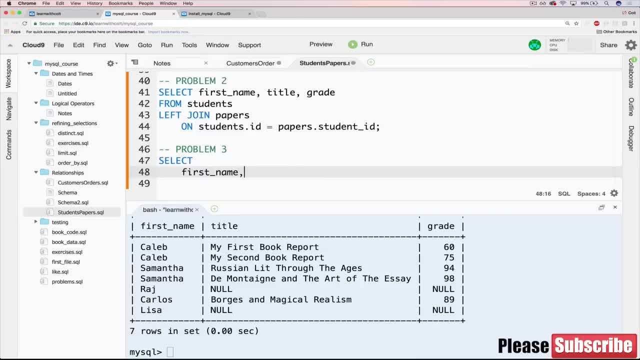 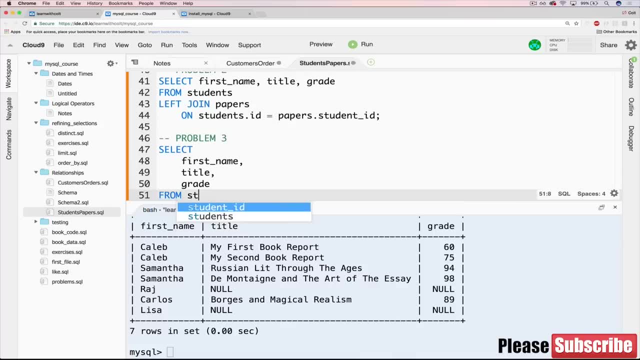 I'll do this on separate lines: first name, comma, title, comma, grade from students left: join papers on studentsid equals papersstudentid part of a mouthful, however, when we're working, so first name will be the same. 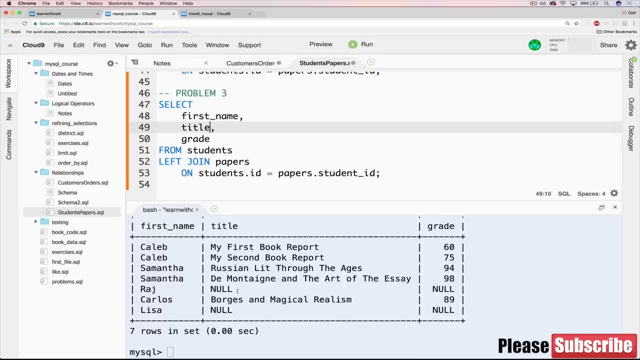 but title we're going to. if it's null, we're going to make it the text of the string missing. and that's where our lovely if null function comes into hand or comes handy, let's say so comma and we'll just replace it with missing. so remember beating a dead horse, hopefully. 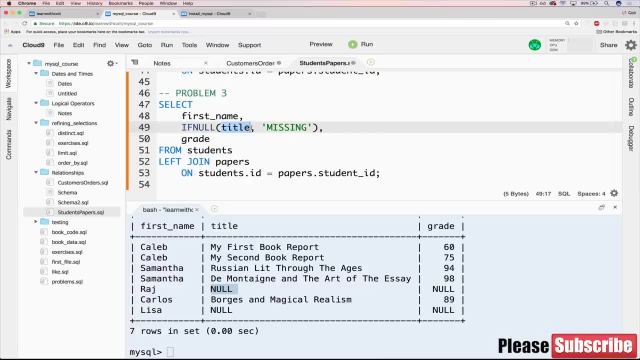 at this point. If null takes this, if title is null, then it replaces it with missing, Otherwise it just keeps it as my first book report, my second book report and so on. So we'll start with that. You can see, we get. 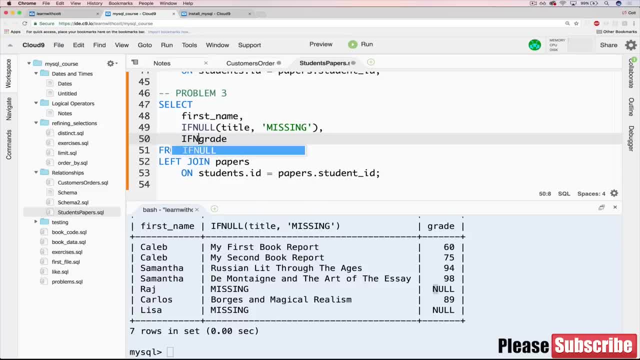 missing. We still have null for grade, and that's a simple fix. The same thing: If null grade comma and we want zero, Not text, not a string zero, We want the number because this is an int over here. Perfect, And we're done. We get missing zero, missing zero, and then things. 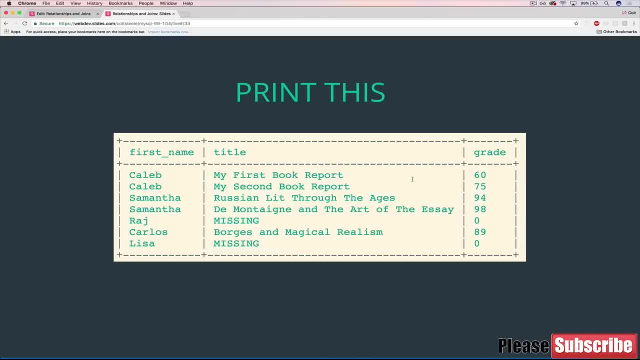 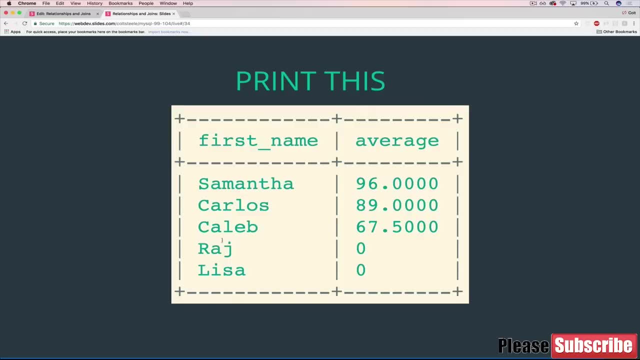 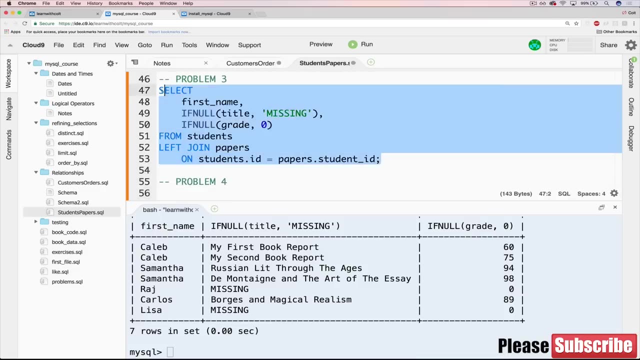 that didn't have null are untouched. All right, moving on, This one is similar in that we want to have data for students who don't have papers. so Raj and Lisa. So this is not going to be an inner join. We know that because if we did an inner join, we would only get these three. 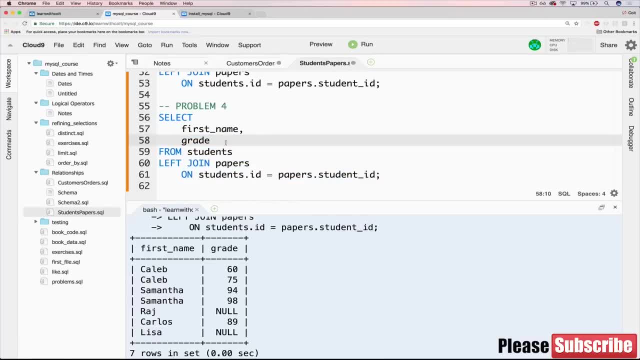 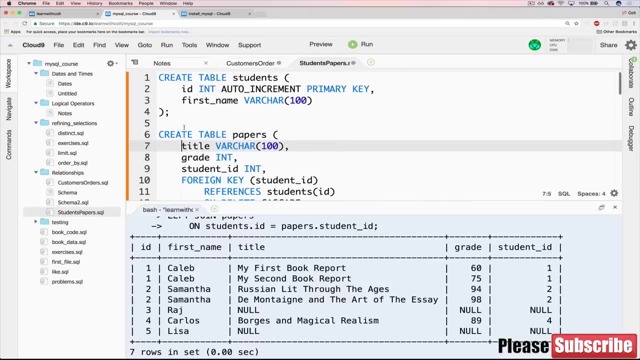 We would only get these three, We wouldn't have anything on Raj and Lisa, Our students who maybe aren't doing so hot, they're not turning things in, But what we want is only the first name and their average for all their papers, And if they didn't turn anything in, their average is zero. So what this really? 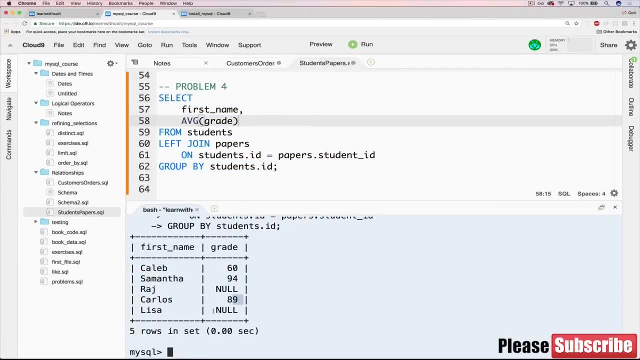 means is we need to group, We need to group our students, And we're going to start by selecting all of this and we'll get rid of our if nulls. So let's just do title again. We don't even need title, do we? We just want grade. 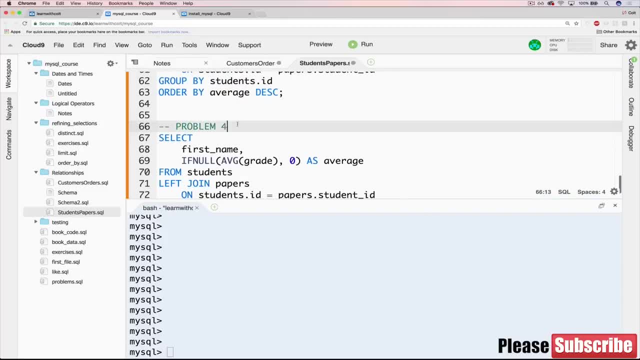 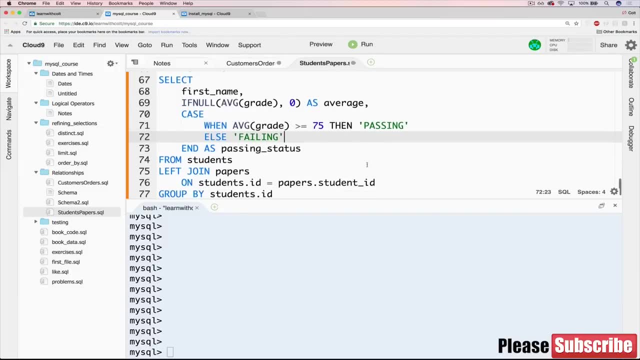 We'll start with that. So if we do a left join, okay, we get this. This is actually close right. The only thing is we need to condense our data. We need to group these together. So what's the best way to group them? Well, we could use first name. That would absolutely work. They're unique. 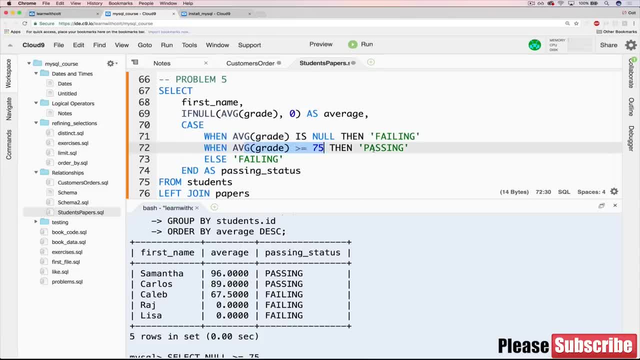 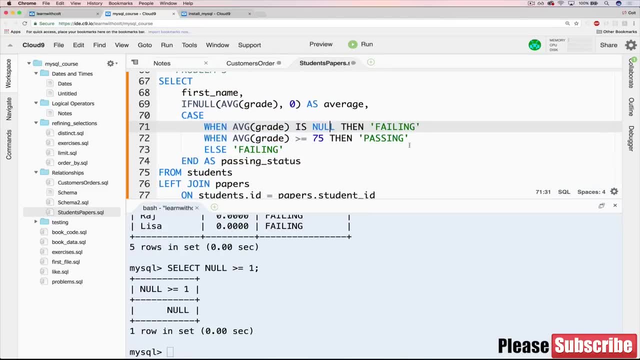 We could not use on the papers side of things. We could not do papersstudentid because Raj and Lisa don't have papersstudentid, So that's null for them, which is problematic. We can't really dependably group by null And also we don't want to group. 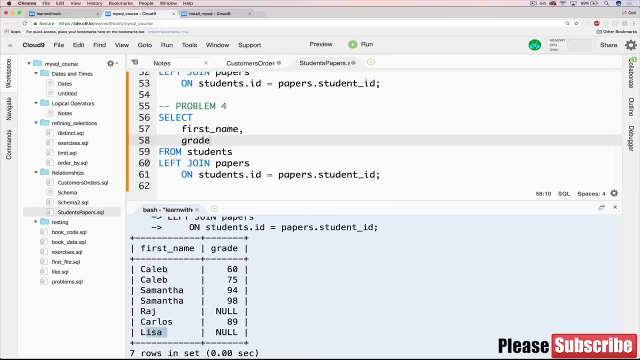 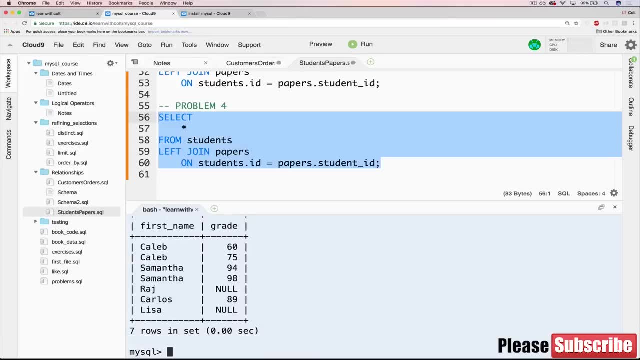 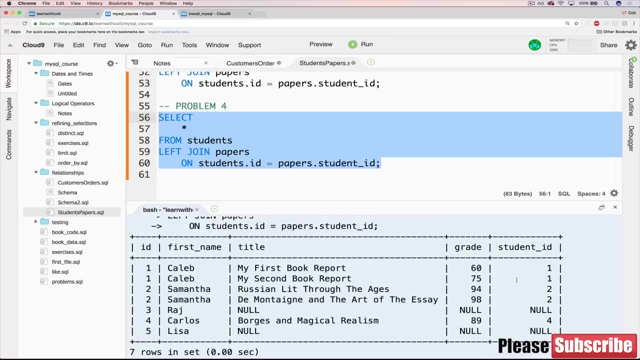 Raj and Lisa together. So we want to group from this side of the table And we could do names, but there's also something else that we're not seeing. If we do star, we can just group by studentid, as you can see here. So what I was saying is that studentid. 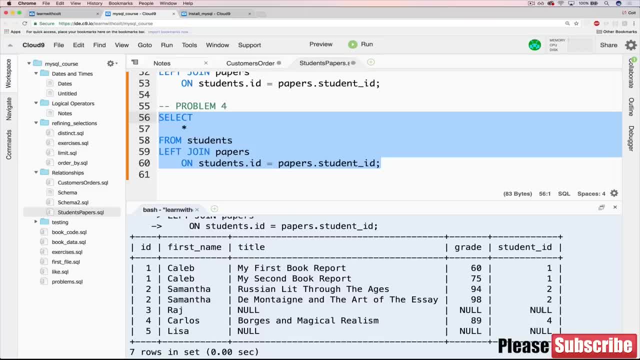 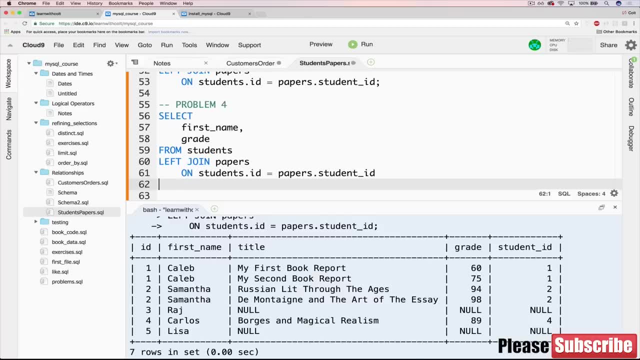 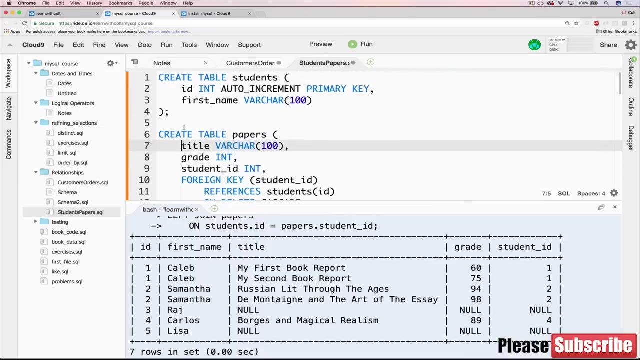 doesn't work because these are null And if we group, we don't want these together, We want them separate. So let's group by students And we could get away with just saying id, because there is no id on our papers. table right, We didn't have id, which we probably should have, just for good. 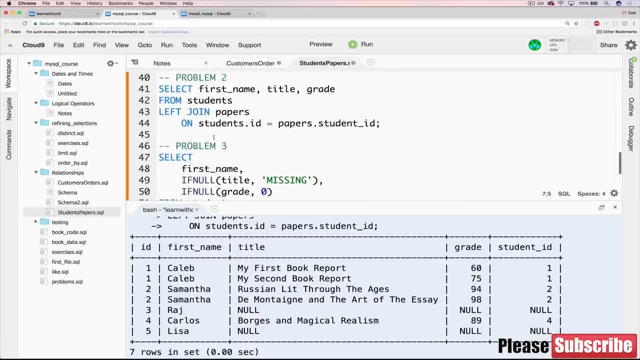 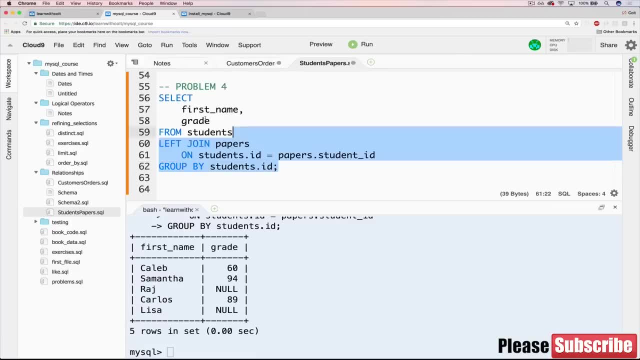 practice but we don't have it. But if we did have it then we definitely need to be explicit and say studentsid, And it never hurts to do that, So we'll group by studentsid And if we copy it and we paste, okay. so we're getting close, sort of We have things grouped. 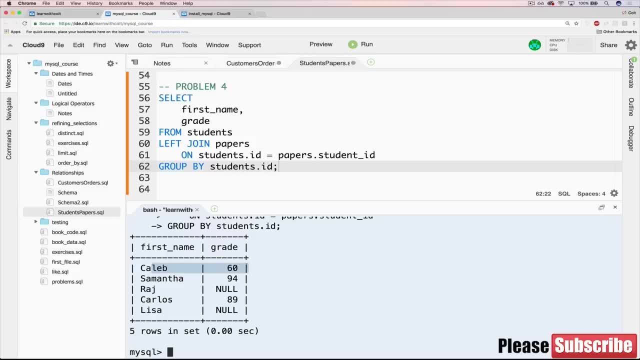 And remember that hides data from us, because it's grouped behind this row: two of Caleb's papers, two of Samantha's, But we're at least getting data grouped. So then the next thing is: rather than displaying grade- here we don't care about grade. What we want to display is the average of. 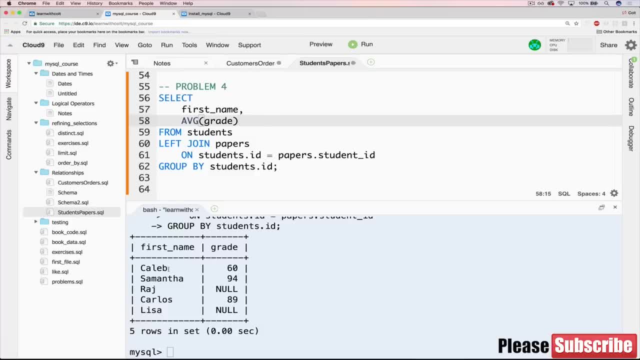 all the grades for those two, So Caleb. and then we have the average of all the grades for those two, So Caleb. and then we have the average of all the grades for those two. So Caleb has two grades- 60 and something else. Samantha has two Raj has. we'll have to deal with that in. 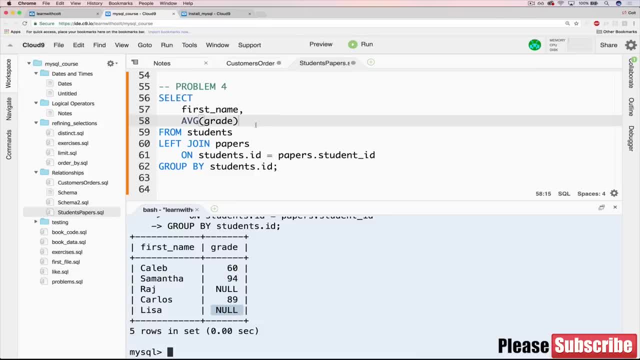 a little bit. Carlos has one, Lisa has null. We'll deal with that in a second as well, But let's see what we get now. Okay, so we get two averages- 67.5, 96, and 89,- three averages. 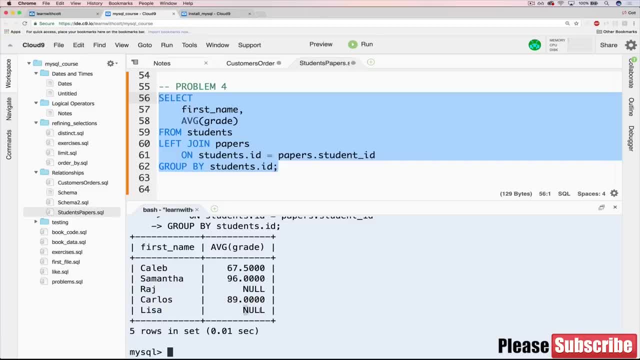 excuse me. And then for our people who don't have papers, we end up with null and null, Simple solution: If they don't have any papers, we just use if null, if null average grade, then we just want to make it zero, Just like that, before I deleted it. 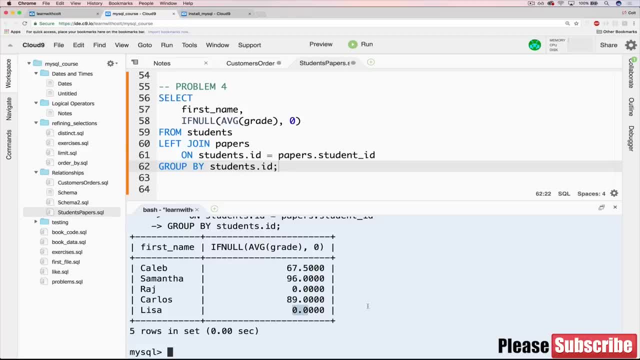 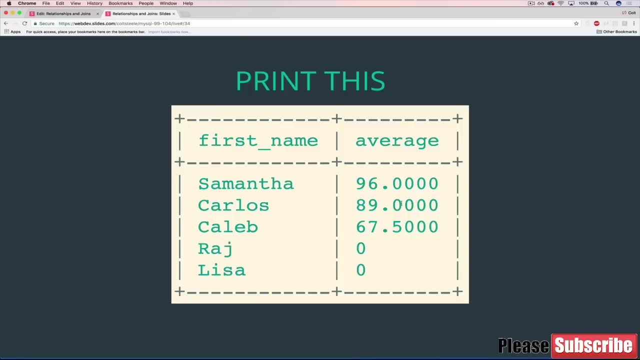 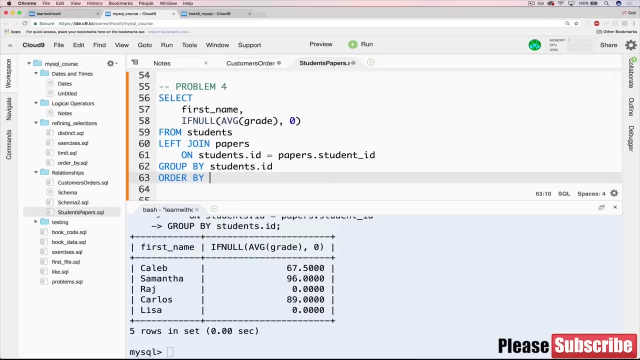 And now you can see we get Raj and Lisa have zeros And if we check against what we had here, there's only one small change, which is we need to order them Descending order by order by average grade. So if we check against what we had here, there's only one small change. 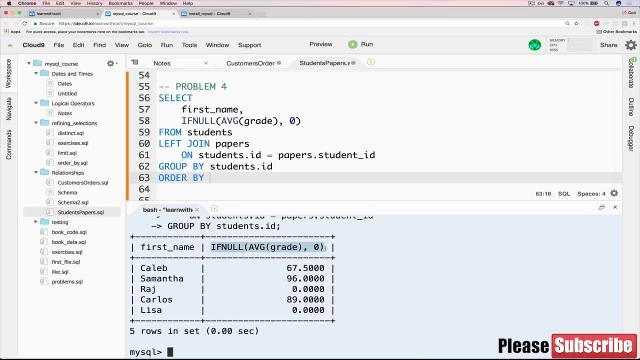 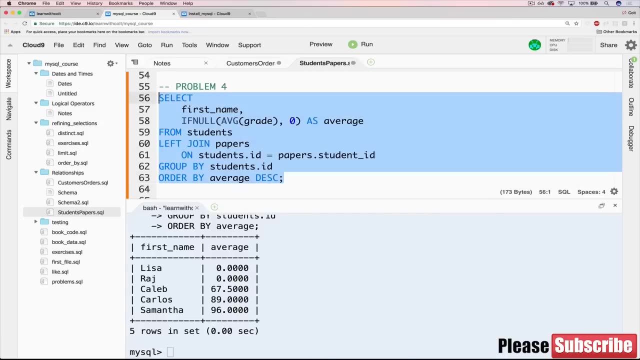 and actually, rather than doing average grade, let's just give this an alias, which is what I did over here. I just called it average. Now we can do order by average, Perfect, And there we go. Well, nope, I lied, Order by average. 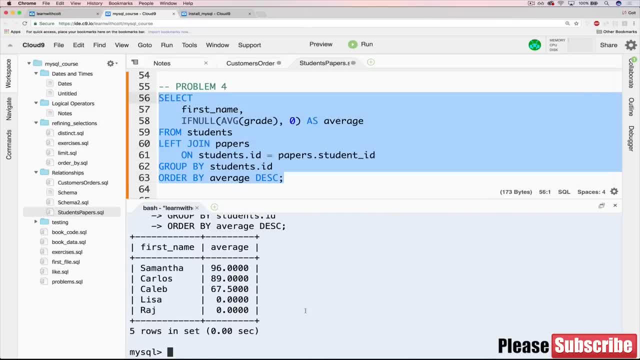 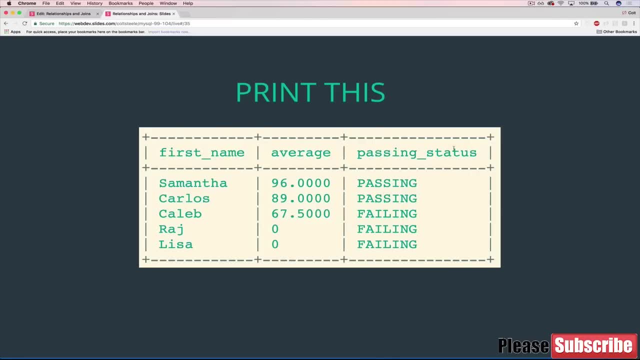 descending. And now there we go. Okay, perfect, Moving on Our final problem: Same thing, although we're just now adding a passing status, So a new field that doesn't exist in either table and that says passing if the average grade is greater than 75, or equal to 75. And failing. 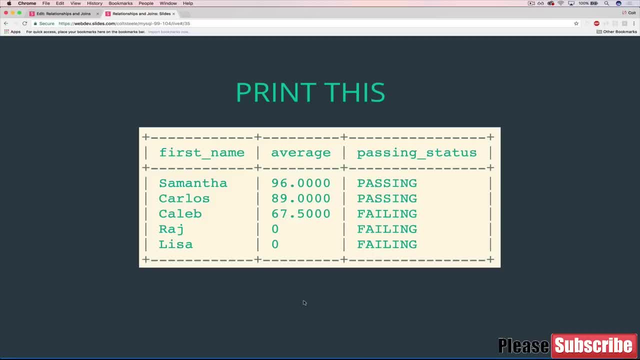 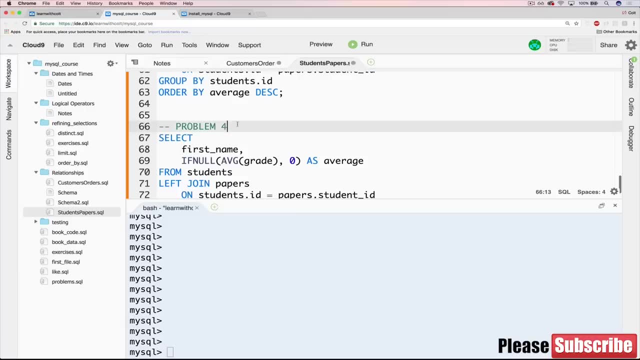 if it's less. So this is a great use for a case statement. Okay, so let's give it a shot. This one is very similar to the previous problem, So I'm just going to copy it, paste it and just rename it. problem five. So all we need to do is add in another field: 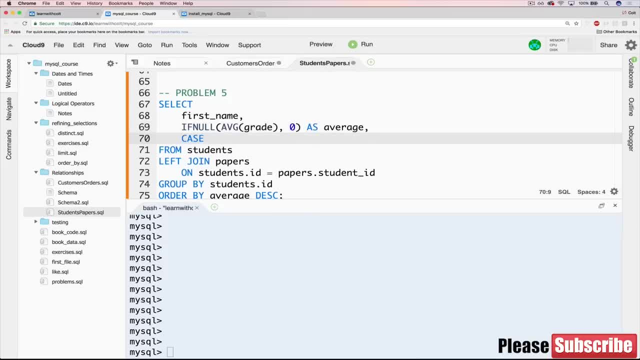 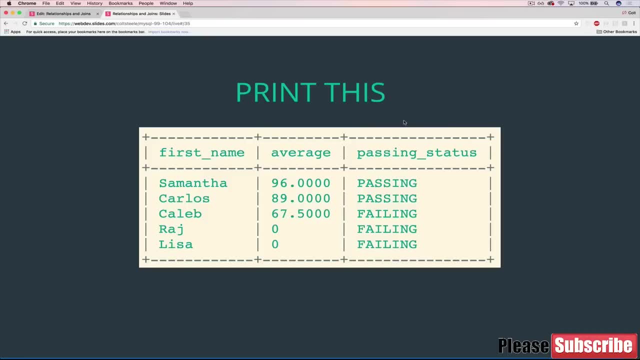 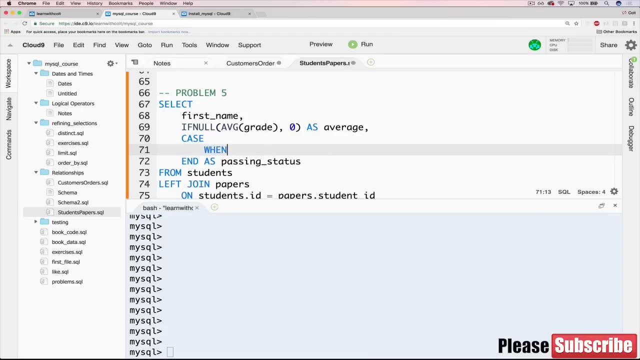 But this field involves a case statement. So what I like to do is always do my case and end together, case end and we'll call this passing was a passing status. there we go, okay. so what do we fill in here? we're basically trying to say when, what, when, average. 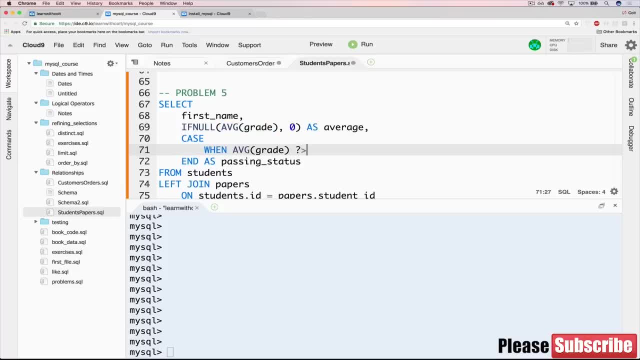 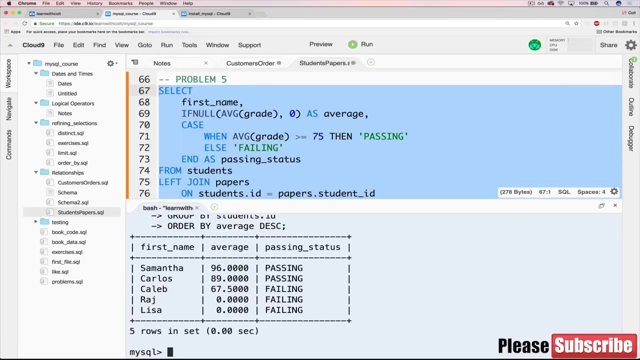 of grade. so we'll copy that is greater or equal to 75. then what do we want? we want it to be passing perfect, otherwise you want it to be failing, and let's see what happens. okay, so it seems to be working: passing, passing, failing, failing, failing. 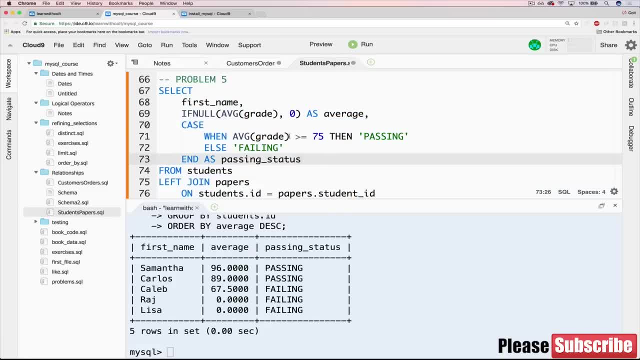 one thing to note, though, is that when we're doing average grade here, for some of them it's null. remember that, and so it's important to realize: if we want to do that, we want to say: if we want to do that, we want to say that we want to add a. 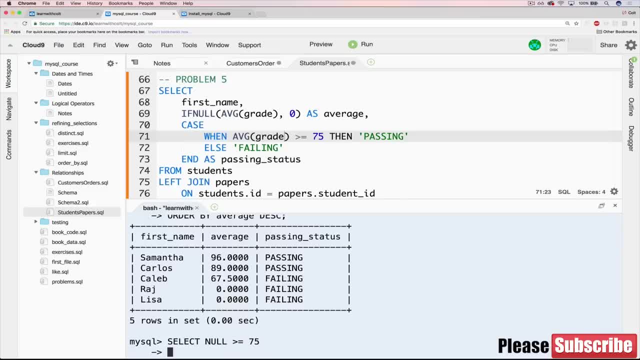 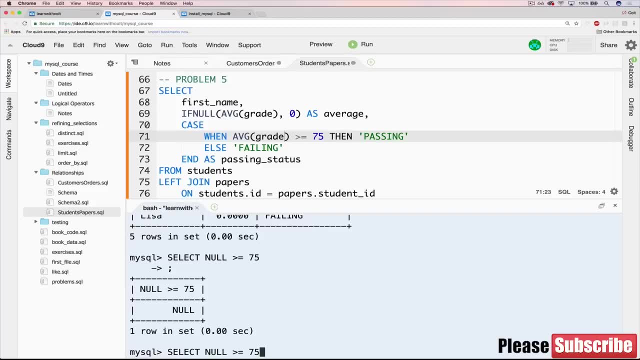 to the queue. so when we say we want to do that, we want to say that we want to do that. we want to say: worked with null. is null greater than or equal to 75? and the answer is null, which is bizarre, right versus if we had done. is 65 greater than or equal to 75? we get zero or one, true or false, but we're. 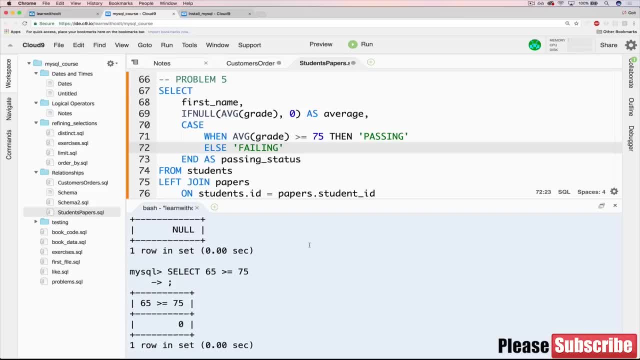 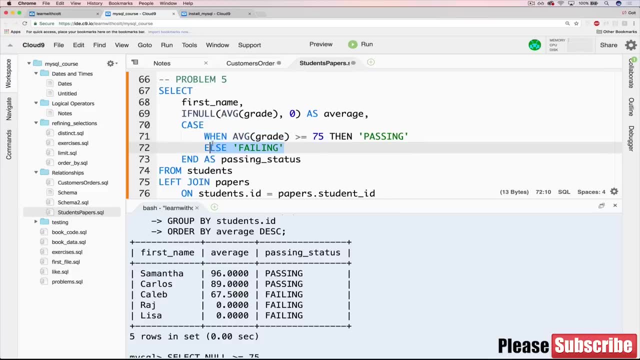 getting null when you work with null. fortunately, that is working to our advantage, because when we get null here, it basically the case statement moves past, it ignores it and does the else. but it is important to understand that. so you could do something like this if you wanted to. 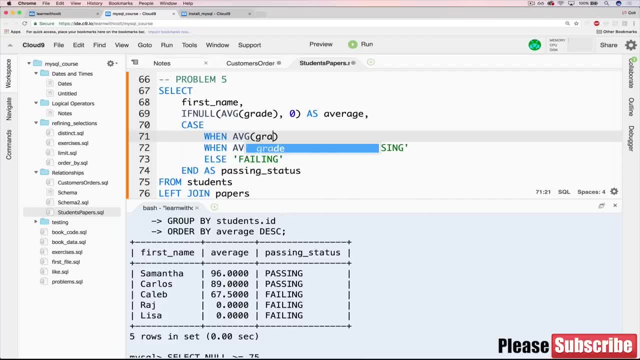 be extra careful: when average grade is null, then failing. so that would catch null right away. then we have okay. when it's a number greater than 75, equal or greater than 75, then passing okay. otherwise that means it's a number that's less than 75 and that means failing. so we won't see. 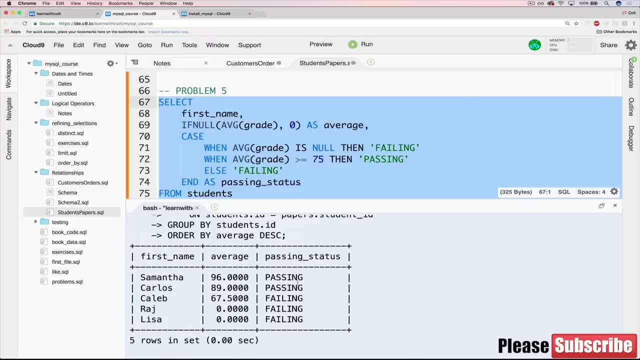 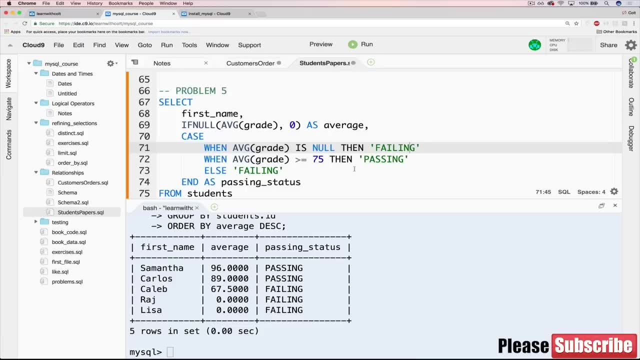 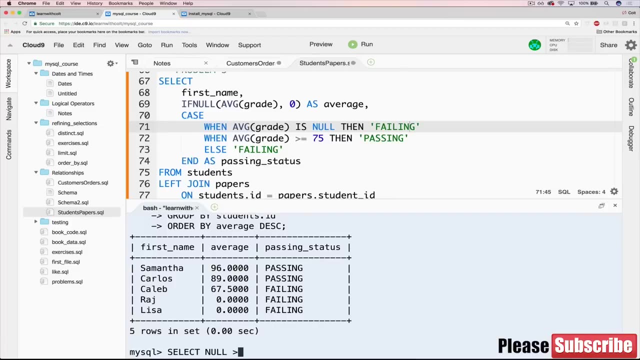 a change in our results here. right, it looks exactly the same: passing, passing, failing, failing, failing, passing, passing, failing, failing, failing. the difference is that we're not relying on this weird comparison between null, because it is bizarre. is null greater than or equal to one? and it tells us null. it just is useless. null is a. 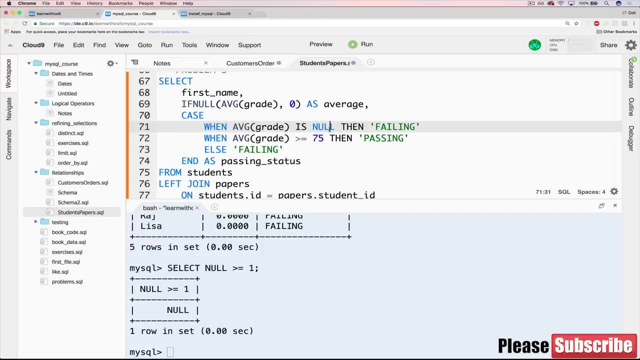 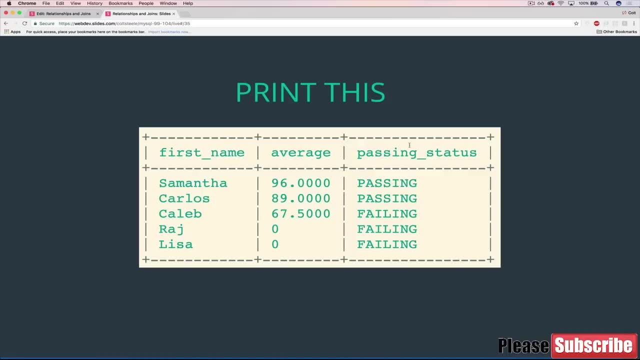 weird special value it has, things like is null, so let's take advantage of that just to be safe. all right, now we're done. hopefully you enjoyed some of that. um, it's a little bit different than some of the exercises we've done in the past, involves joins, but hopefully it's not too scary. 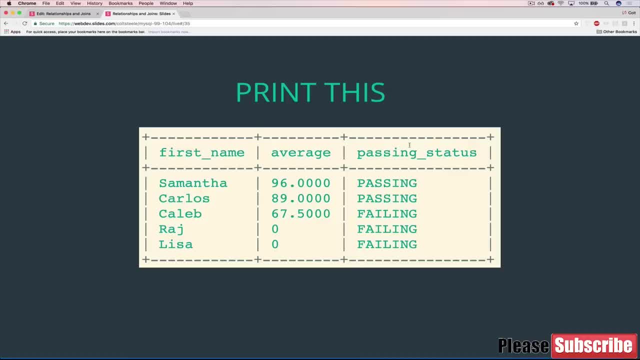 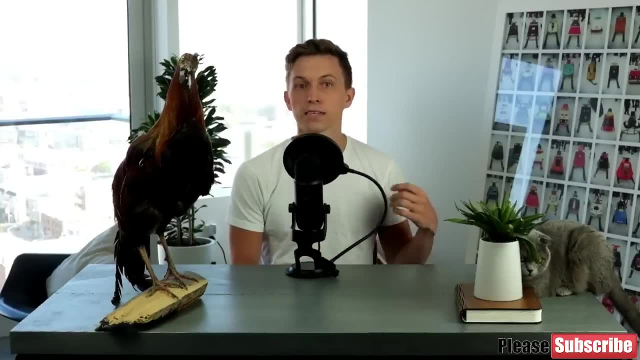 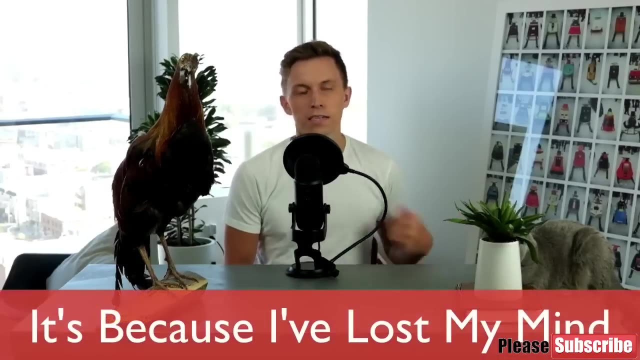 and if it is, i'm sorry. just i'm sorry, hang in there. hey, welcome to the next section. so i'd like to start off this section by asking you a question. it's not really a quiz or anything, but i just want to know why there's a chicken on my desk and, in the meantime, blue and i are here to 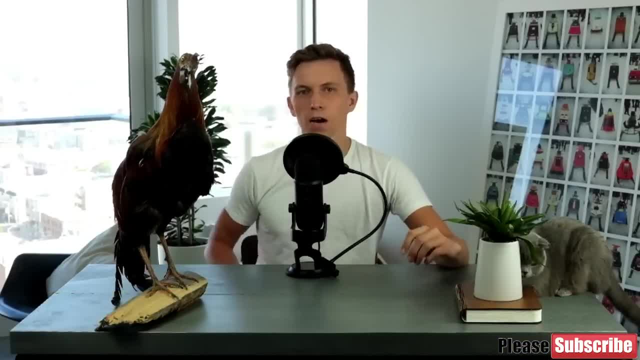 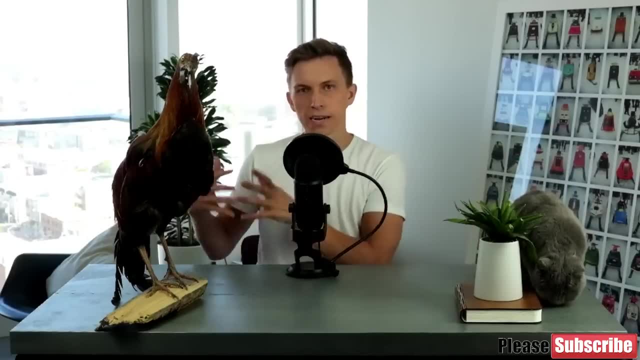 talk to you about the next section. so we're continuing on our trend of working with multiple tables. we saw a one-to-many relationship in the last section. now we're moving on to a many-to-many relationship and i saved this one for second. it's a little more complex, don't be afraid, it's still. 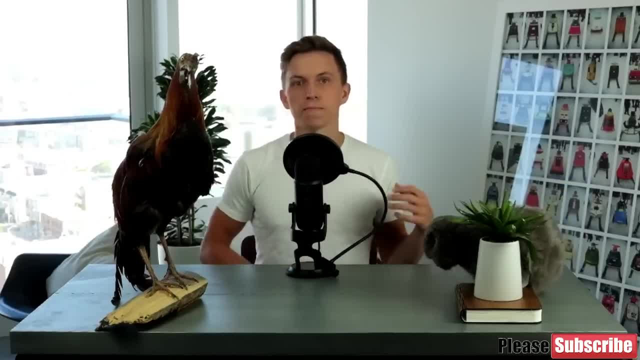 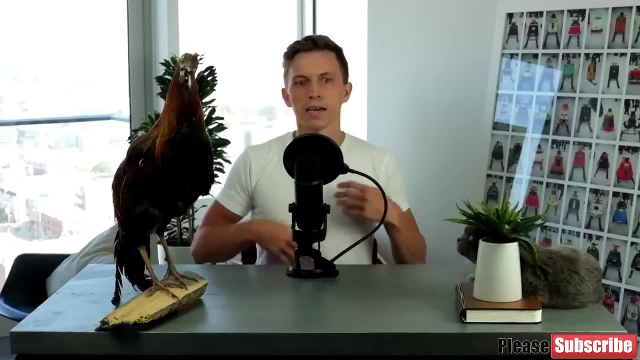 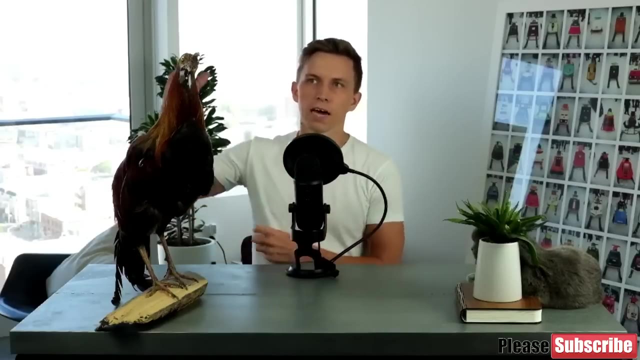 very doable and very important. i keep saying that- very useful to be able to have multiple tables with a many-to-many relationship. so we're going to focus on this section on implementing a schema for tv shows with reviewers and the reviews that they write. so think of, like i don't know, breaking bad. 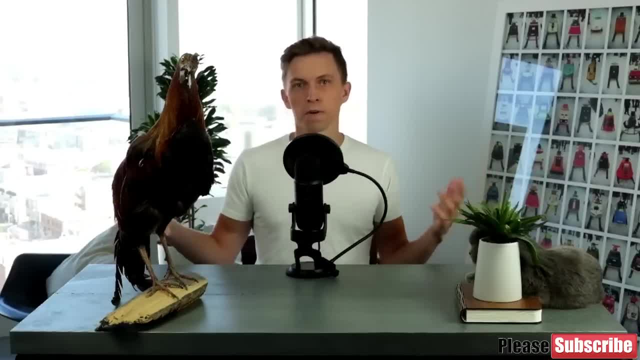 and american horror story, or two different shows. we'll have a bunch of them. i'll give you data- and then 10 different human reviewers, maybe a cat or two as well, and these reviewers can go and assign ratings to every show. so i could say: this is a 10, that's a nine, that's a four, whatever. 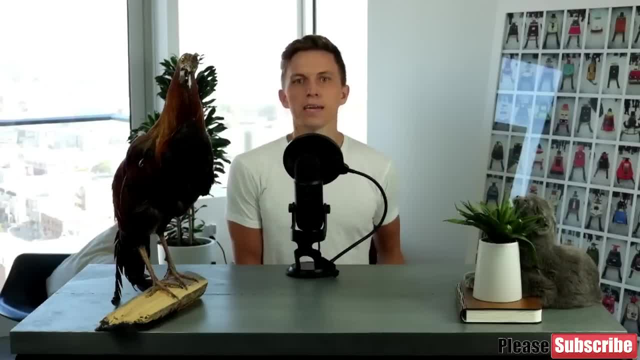 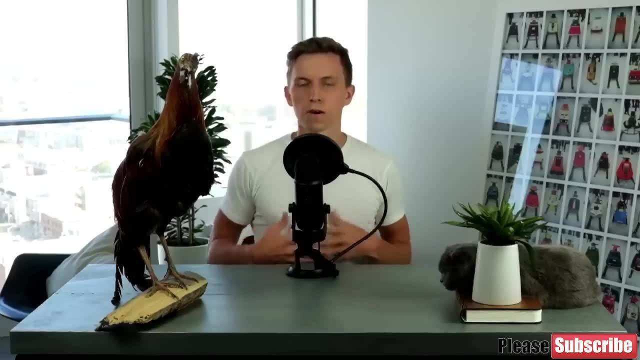 uh, so that's what we're going to implement: that sort of a schema which is a many-to-many relationship. hey, hey, stop eating that, eat the chicken. so okay, where was i? um, exercises: yes, this section is all exercise. basically, the way that i decided to do it is to go through. 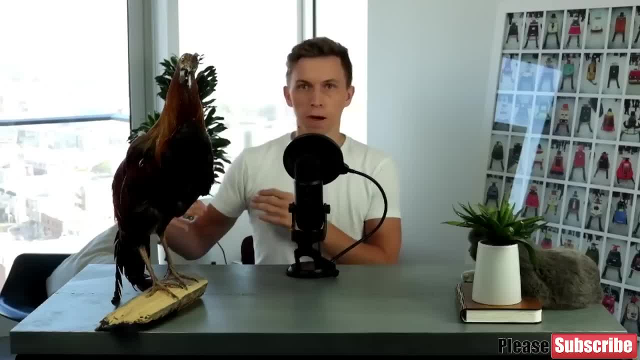 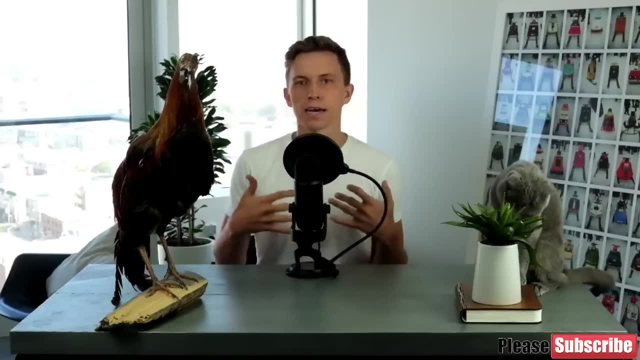 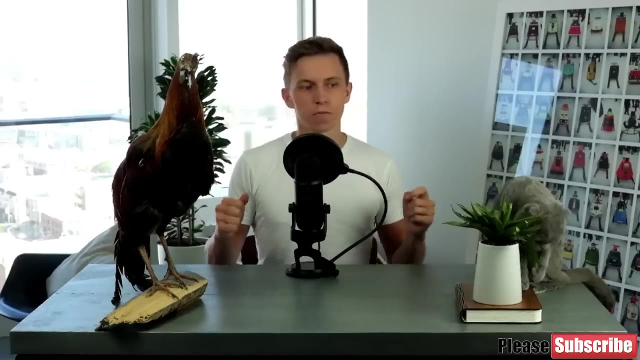 not only building the schema but also asking common questions about the data and performing common operations and the joins we want to perform, basically as we go. so the whole thing acts as a bit of a code along slash exercise. so hopefully you like television. if you don't, then this will be a great insight, great window into the world of television for you. 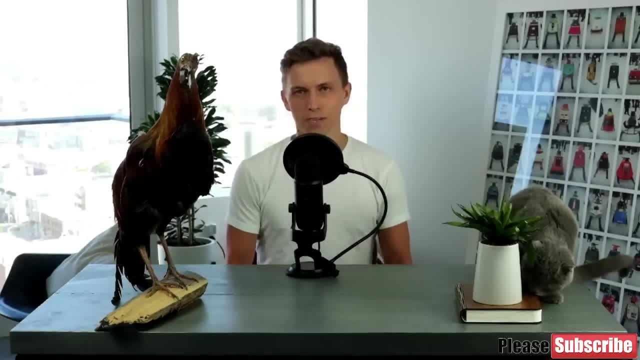 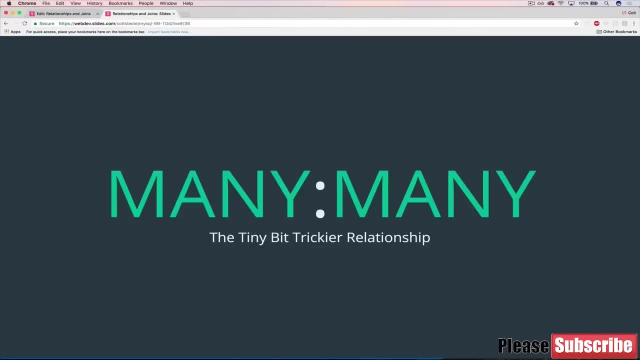 but, more importantly, we're talking about joints, again, working with multiple tables. all right, all right, welcome to the next section. so we're continuing on the same similar path, talking about relationships, talking about joins, more complex data, multiple tables and connecting those tables, drawing lines between them. however, we're now moving on to our next relationship, which is the many-to-many relationship. 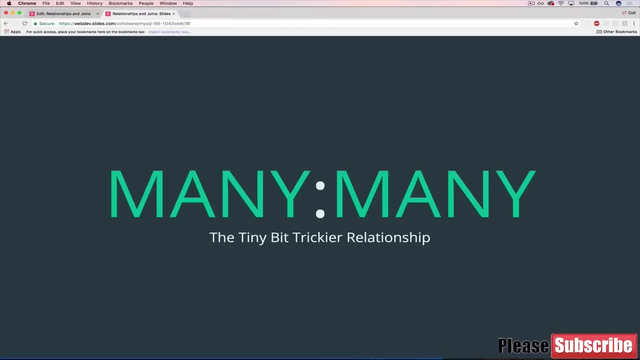 so we saw how to do a one-to-many, which is a pretty standard relationship and it's pretty common. many-to-many is is common as well, maybe not as common, but still very, very common. so we're going to see how to do it, and the reason that i saved it for last is that it's a little bit trickier. 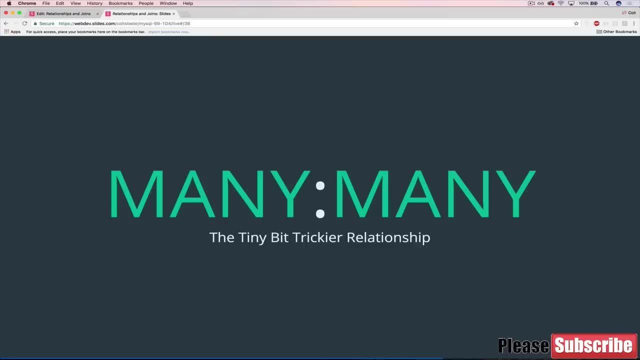 it's not hard. i don't want to scare you away, but you'll see there's a little more setup involved and then, once we've discussed how to use it for each problem, then we find the answer and we estimate how it's subscribed and then we spend. 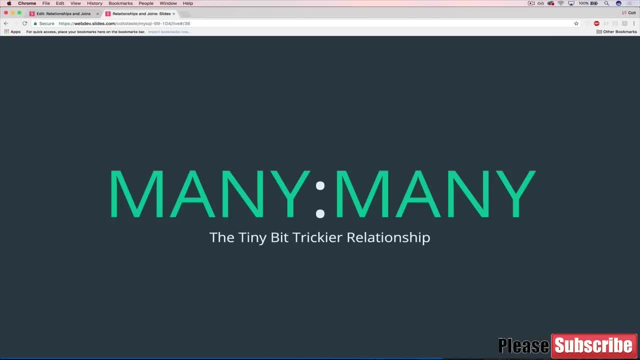 along with what we can, and then we do some coding. so i TU, I'm going to use some relatively complex data that i've spent way too long creating, and then we'll do some problems together. so this section will actually serve more as a code along. so i would encourage you, if you don't, 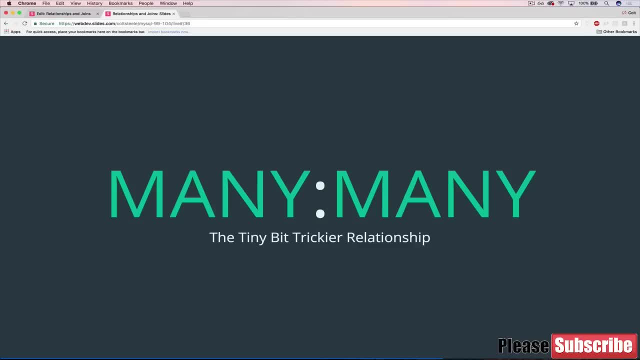 typically. i encourage you to follow along. we're going to use some relatively complex data, like i said, and we'll just go through it, do a couple exercises together on a many-to-many relationship. so let's start in this video just by talking about the many-to-many. 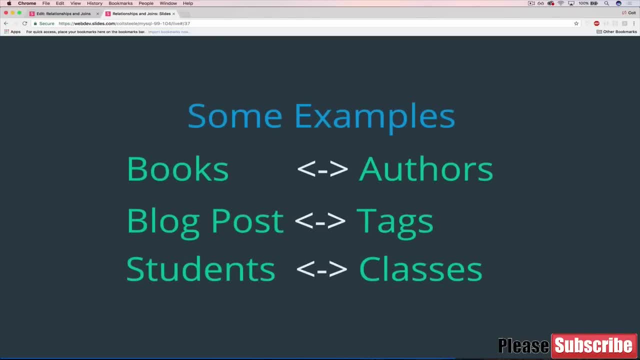 relationship. so we kind of discussed it briefly in the last section, but here are a couple examples. so books and authors. hearkening back to that last section where we saw books, a book can have multiple authors. right, there are lots of books that are written by co-authors or teams of you. 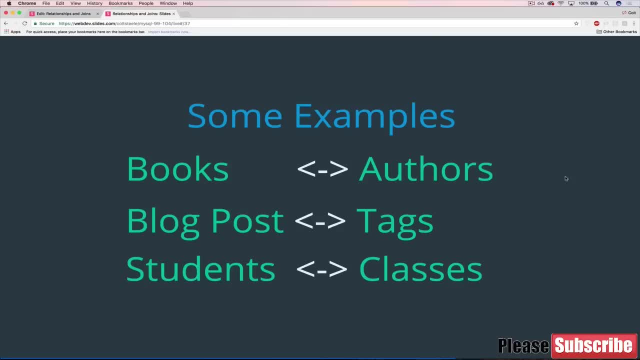 know if it's a collection, if it's an anthology, there might be 20 authors, and each of those authors can then have multiple books. so it's a many-to-many relationship. books can have many authors, authors can have many books, or another common example is blog posts. 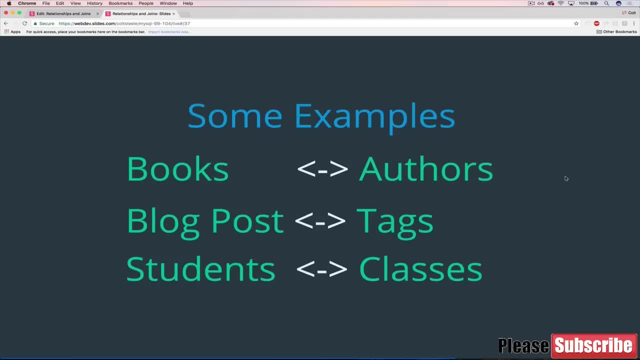 or some sort of content, whether it's an instagram photo, a tumblr, whatever you call it, a tumblr post, you know, or just a traditional blog- some sort of content and then tags. tags by that i mean things like, um, you know, sunset picture, or uh, there's some really so like. 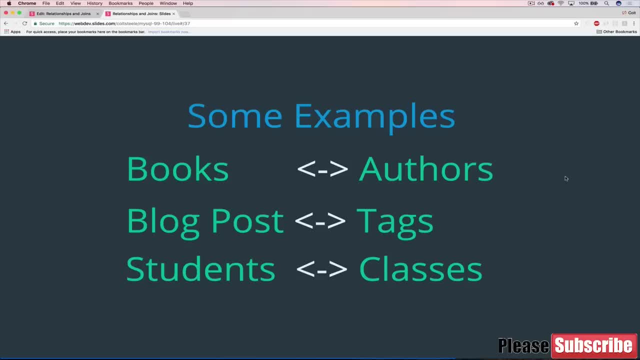 van life, if you're familiar with that hashtag, or i do a lot of photography, so i see a lot of tags that are things like um, like masterpiece landscape photography, and then um, you know insta- good, if you use instagram, there's all these different tags that are out there. 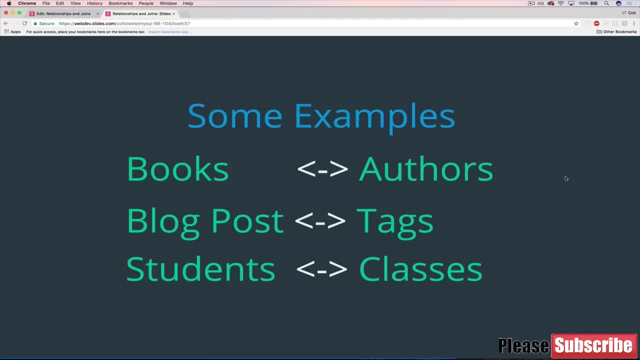 and each post can have multiple tags. i mean, there's a limit sometimes, but you know, on instagram you can have 30 hashtags- i think it is on a photo- and then each of those tags can then have as many posts or photos as necessary. so that's another example, and the final example i have here is students in classes. 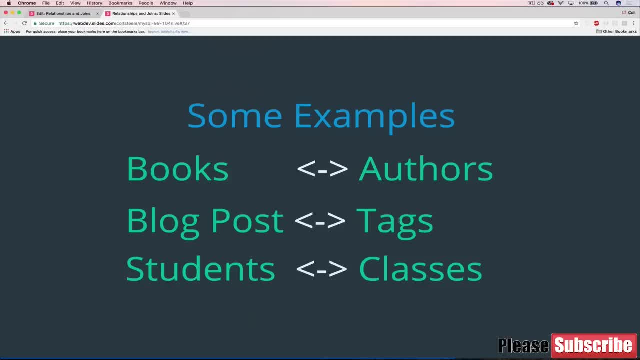 so this is we're talking about, like maybe college students or university students, where students have multiple classes. they pick their classes at the beginning of the semester. one student can have usually each of the four tags on their instagram resume, or even regular must have multiple classes, unless maybe it's your last semester but you have multiple. 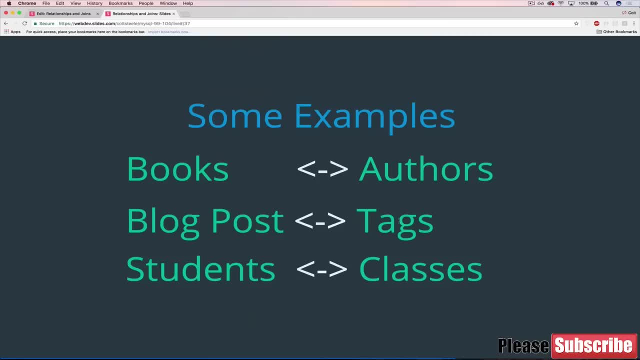 classes that you go to, that you're related to, and then each class is going to have multiple students in it, and that's a many-to-many relationship, and the one that we'll be working with in this section is actually not listed here. it's a little different and, to start, 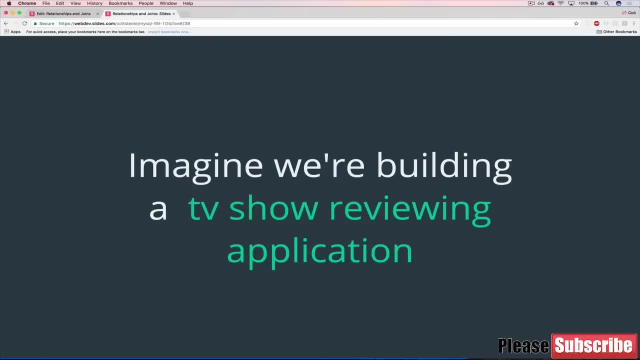 off. I want you to imagine that we're building a TV show reviewing application like: yes, I know we don't need any more of those, but imagine something like Internet Movie Database- very, very simple version though, but we're working with TV shows exclusively, and the 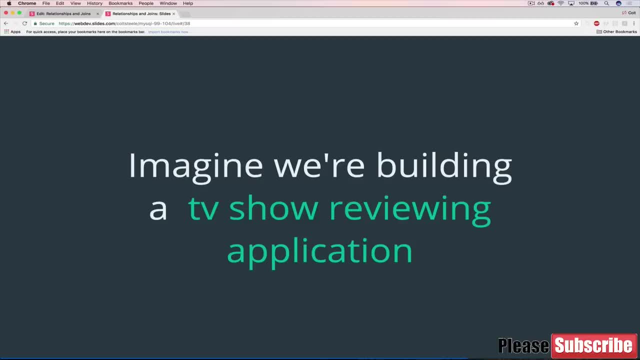 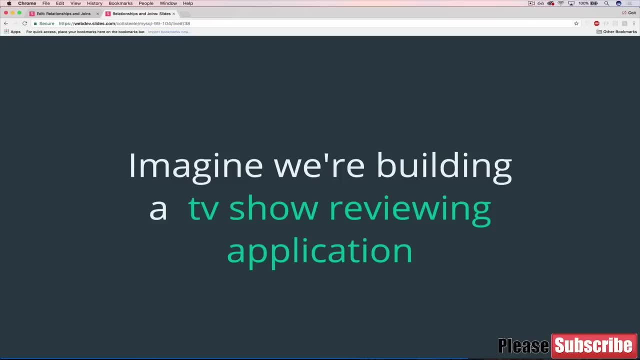 to accomplish this relationship, a many-to-many relationship, where we're basically associating users or reviewers- we'll call them- with TV shows, we need to actually use three tables. We use what's known as a join table or a union table, so we have our series data up. 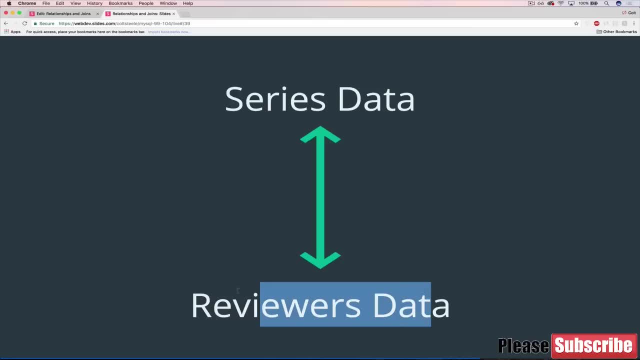 here, so these would be the TV shows, and then down here we have our reviewers data, so these would be just names. in our case, we'll keep it very simple: this will be Colt or this will be Charlie. 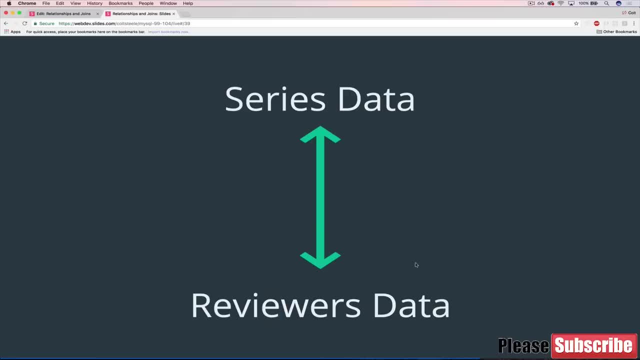 or whatever it is, but the way that they're connected is through a third table, through a reviews table. so this will make sense when I show you the schema in just a moment. but think about it this way: series exist on their own, they're just TV shows. reviewers exist. 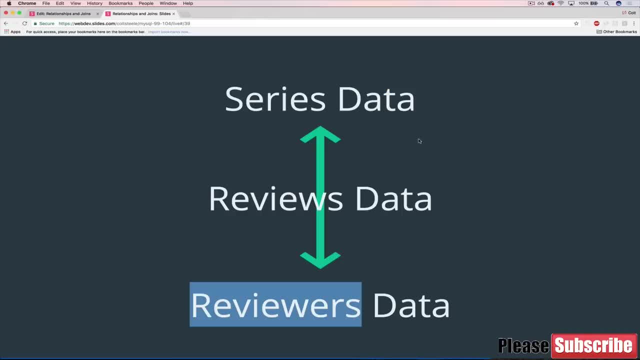 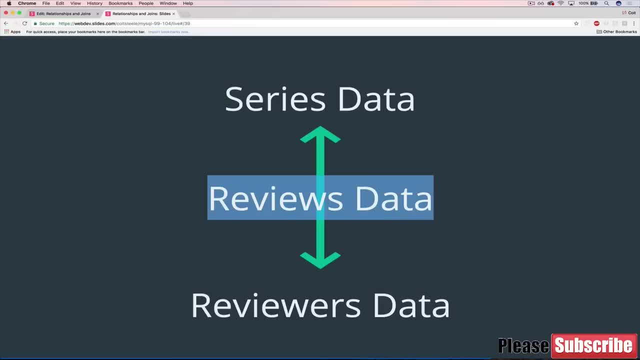 just a TV show, and they're just a TV show and they're just a TV show. So they then are associated through this reviews table. so this reviews table will have information on the TV show that's being reviewed and then the reviewer who is doing it as well. 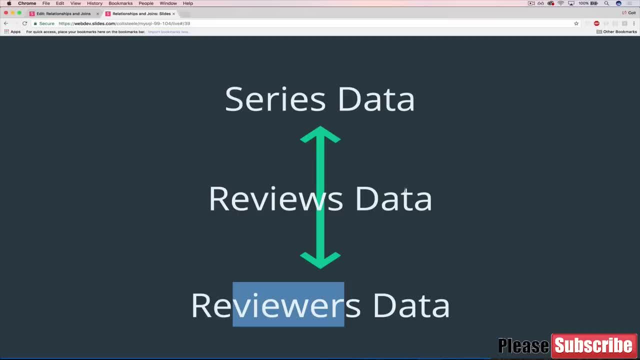 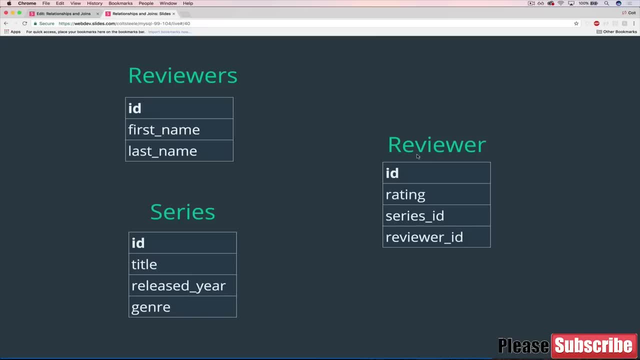 as a third piece of information, which is the rating. what's the number, the numeric representation of that review. So, without further ado, let's take a look at our schema. We have three tables: reviewers over here with an ID, primary key, first name and last. 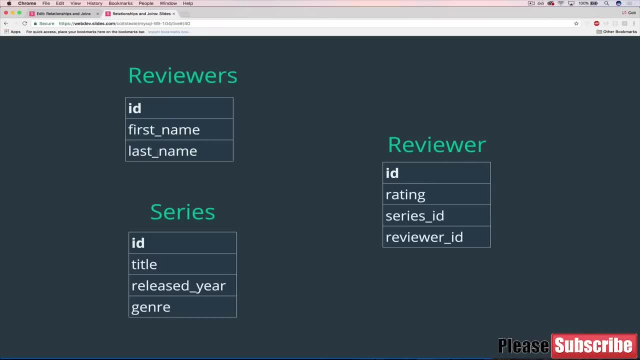 name, real application. we would have more data here, right. We would have email. We'd be storing our password in a safe, protected way. We would have things like registration date, maybe last active, all that kind of stuff. But to keep it simple here so we can focus on the relationship focus. 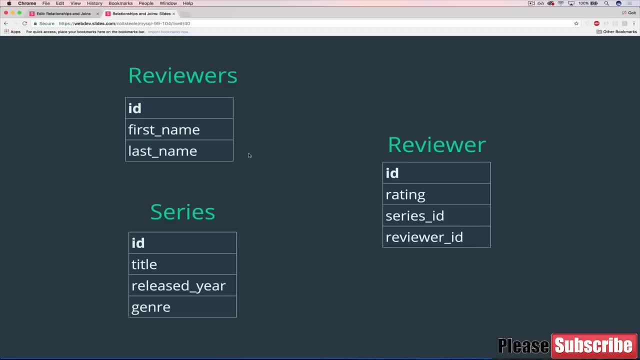 on the joins. I'm only doing first name and last name. Then we also have series And you know this is something I actually debated. The plural of series in English- modern, traditional spoken English- is just series. However, a lot of people would argue that we should name this table. 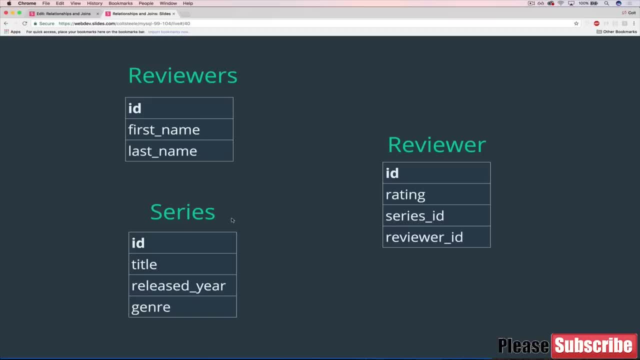 serieses with an ES in the end. just to make it clear that that's the table name. I'm not exactly a fan of that. It's really determined by the project or the team you're working with, or by you if you're working on your own thing. I've worked on projects where we had to abide by that. 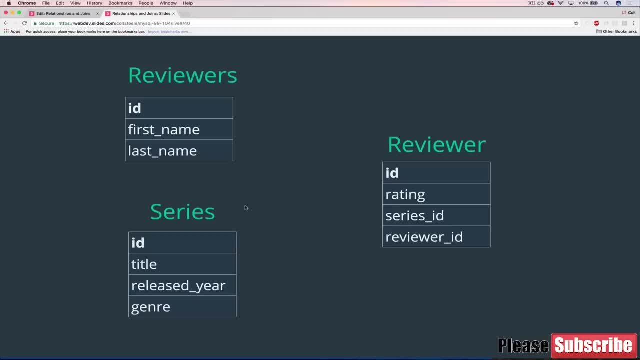 where the plural was always with an S afterward, even if that meant mouses instead of mice. But I'm going to leave it as series, just because I think it's simplest. So series has a primary key ID, a title. so that would be Fargo, which is a TV show as well. Really good TV show actually, not just a movie. 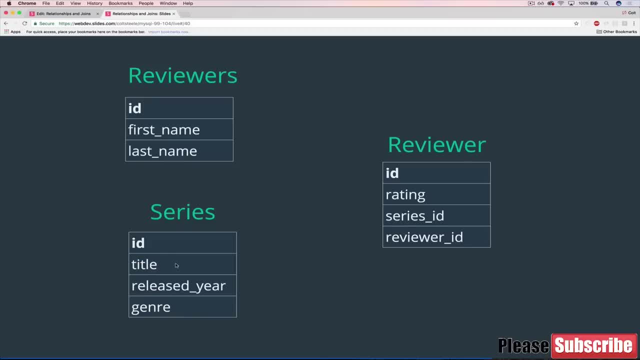 So Fargo or Halt and Catch Fire, Seinfeld, and then the release year, So 2014 or 2002, or whatever it is, And then a genre which we're going to keep very simple. We're only going to 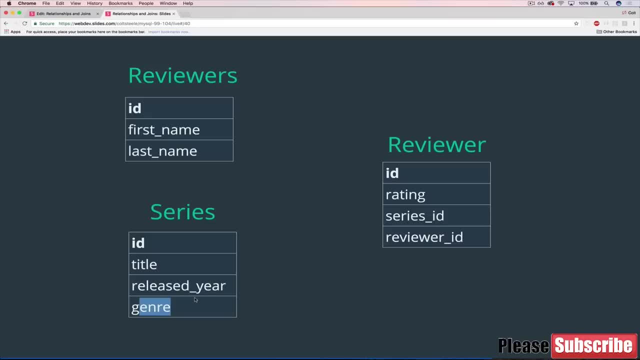 have animation, comedy and drama. So just a couple of examples of genres. But again, these on their own are just separate entities. Where they're joined is through this third reviews table, which is what's known as a join or union table. 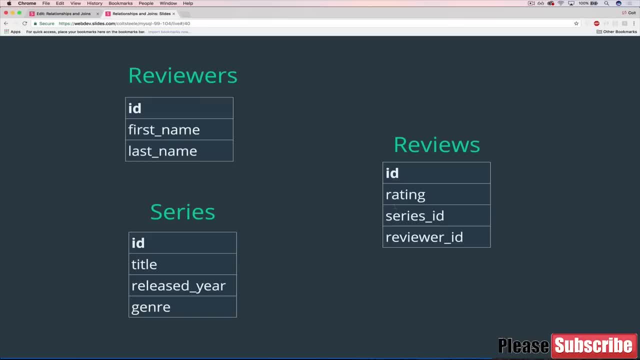 It's connecting these two And the way it's doing that. well, first of all, it has an ID. Nothing special there. Every review has an ID, There's a rating, So this would be 5.0 for a fantastic show. 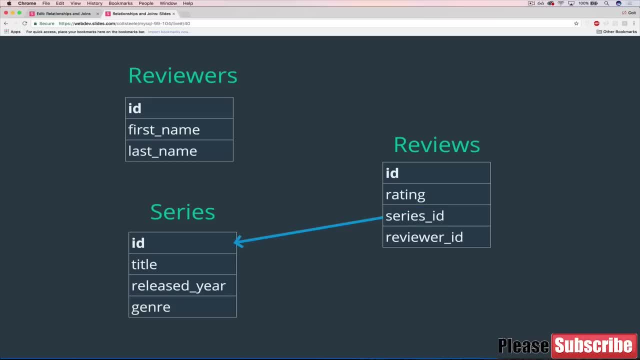 Then the series ID. So that's going to be a foreign key pointing to the series table. So what series Is this Fargo? Is this Seinfeld? And then the same. well, not the exact same, but the same idea. for reviewer ID, It's going to be a foreign key pointing to the reviewer's table. 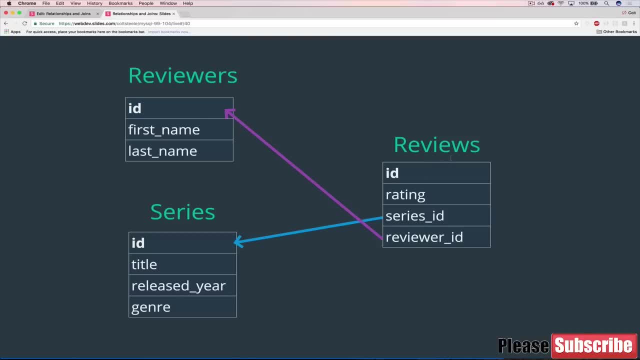 the ID field. So then a single review will have an ID. It will have a rating 9.0, a series ID like 1, and then a reviewer ID, Which could also be one. They're pointing to different tables, So this is a centralized. 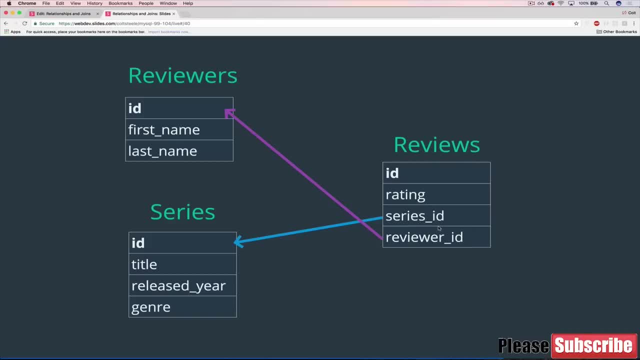 repository or centralized place for our information to be stored. It's connecting these two tables through this table, So hopefully you can see how this is going to work Basically. reviews on its own is going to be a pretty ugly table to look at. It's just going to be numbers. You'll have an ID. 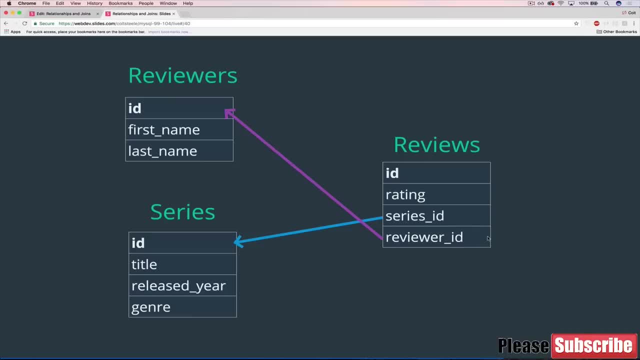 which is a number, Rating is a number, Series ID is a number And reviewer ID is a number. So looking at it on its own is actually going to be very confusing. It's not going to make sense, So we'll have to use joins. 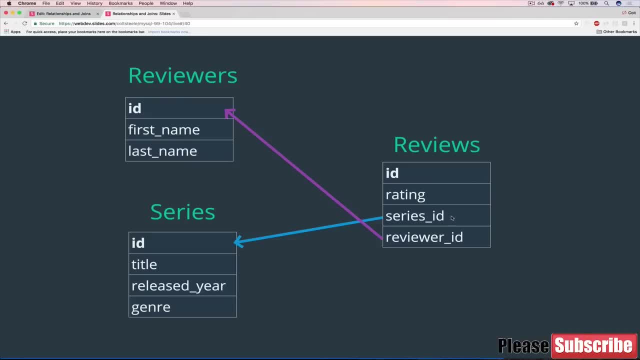 to be able to understand things, so that we could use a join to replace series ID with the name of the series, so that it says Fargo instead of 1. Or it will say Blue Steel instead of reviewer ID 3, and so on. So that's our basic idea here. Here's an example with some simple 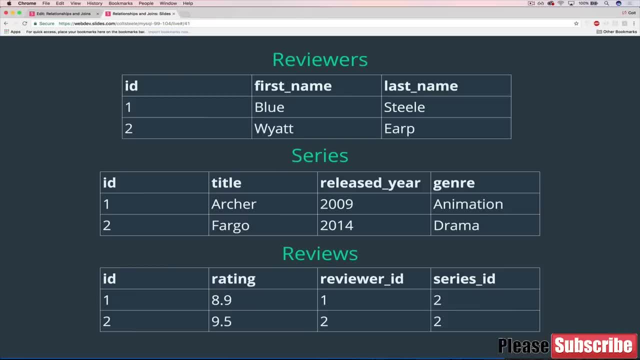 data: Very, very simple. Two reviewer IDs. So we've got Blue Steel and Wyatt Earp ID of 1 and 2.. Then we've got two series: Archer and Fargo. If you're not familiar with these shows, don't worry, That's not. 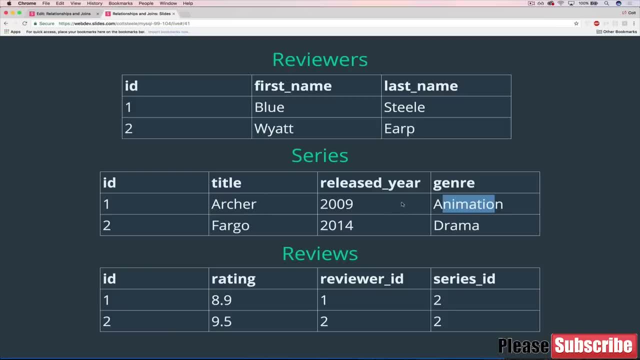 necessarily relevant. Archer is animation, released first in 2009.. Fargo is a drama with a little comedy, released in 2014.. Archer has ID of 1.. Fargo has ID of 2. So they're independent. But then our reviews table. Well, somebody reviewed something. 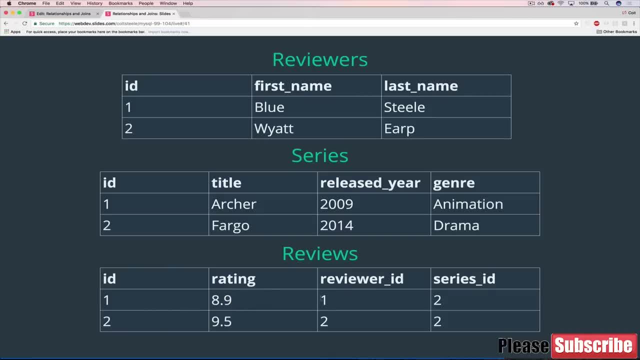 with a rating of 8.9.. The person who did that has a reviewer ID of 1. So that is Blue Steel. So Blue Steel reviewed something and gave it an 8.9.. Well, what did she review? Whatever has series ID 2. So Fargo. So Blue gave Fargo an 8.9.. Then we have a 9.5 down. 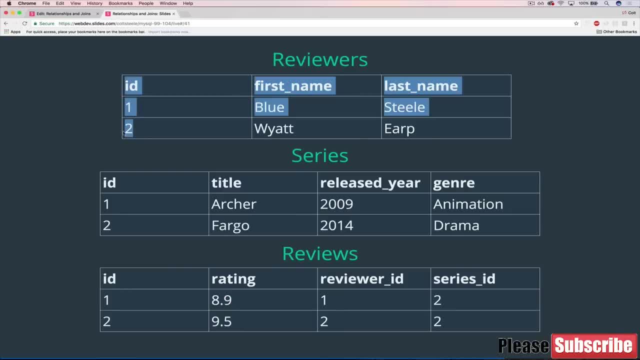 here and the reviewer ID is 2.. So that's Wyatt Earp, this field or this row here in reviewers. Wyatt Earp also reviewed Fargo. This is ID 2.. As we can see, corresponds to Fargo. So essentially what we're storing. 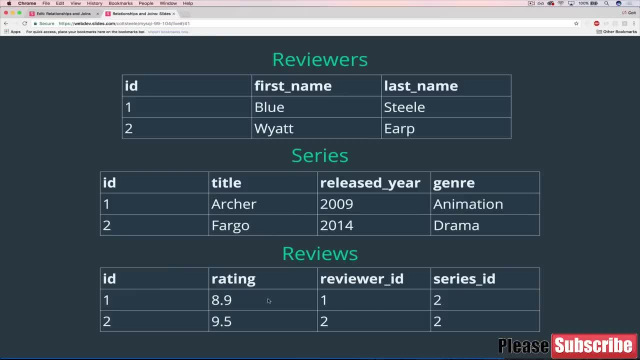 here, Fargo has been rated twice, Once by Blue as an 8.9 and once by Wyatt as a 9.5.. So, as you can see, the data is not that pretty in this table, And this is only with two reviews. 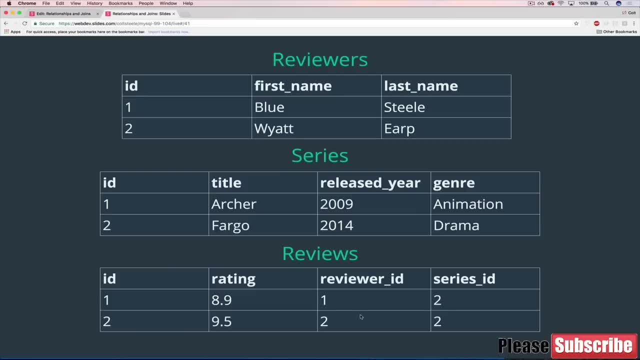 We'll be working with somewhere around 100 reviews, which is a lot of data to look at on its own, And so we'll really be focusing on making that data understandable- readable- which is really the point of this entire exercise. So we're pretty much done here. in this first video, We didn't actually do anything except. 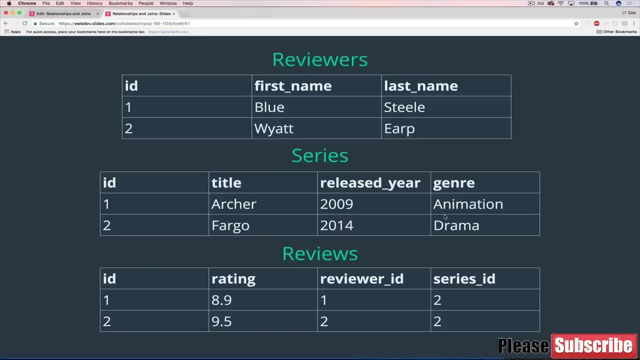 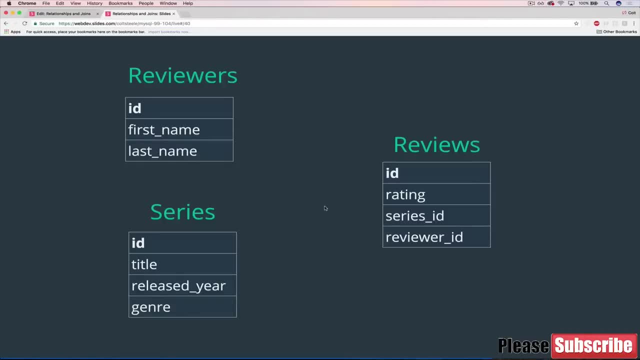 discuss our schema, But in the next video we'll actually go about implementing the tables and inserting some data on our own. All right, So let's hop over to Cloud9 and we'll start simple. Let's work with the reviewers table. It's the simplest one, So we're going to implement. 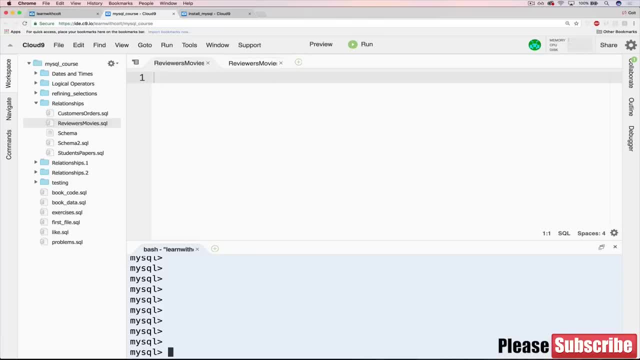 that first. So we'll go over here And, just to be totally transparent, I created a new database just so we have a fresh place to work. You don't have to do that as long as you already have tables named, Series, Reviewers and Reviews. If you do, you may want to make. 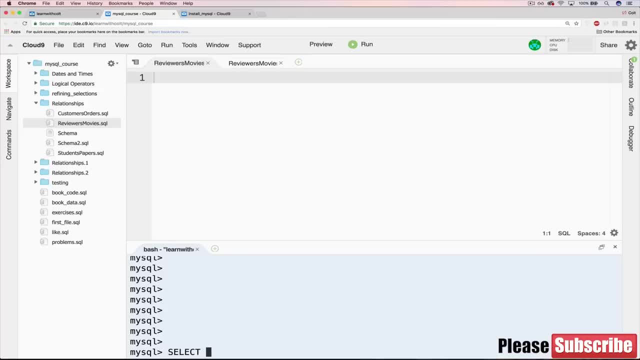 a new database, So I'm working in one called something ridiculous and stupid that I probably will regret: TV Review App. Yeah, not too bad. So we're going to start off by creating a table which we're going to call Reviewers. 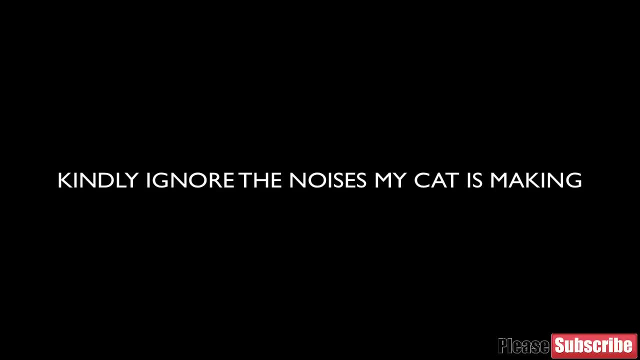 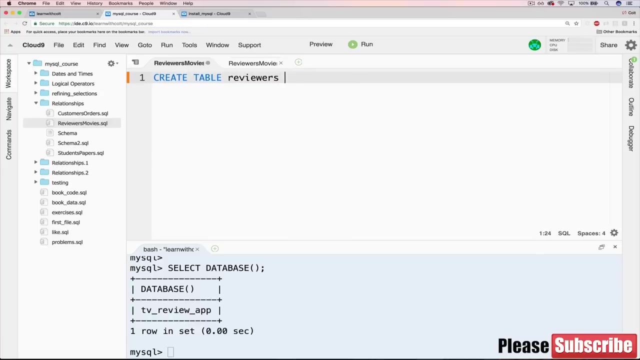 I swear to God Blue, Stop, Calm, down, Calm. So we'll start off by creating our table, which we'll call Reviewers. And Reviewers only has three things: ID, first name and last name. So we'll start off with ID, then. 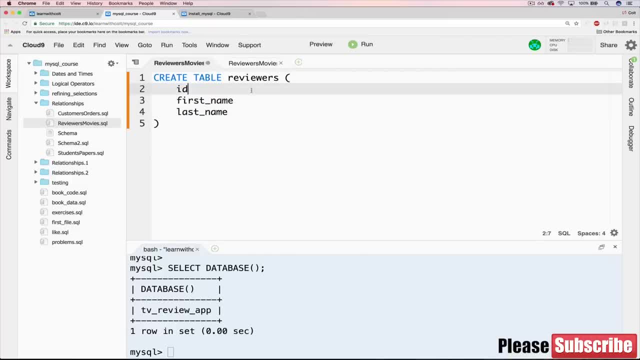 first name and last name, And we know ID needs to be an int. This should be familiar by now. Auto increment: primary key: First name will just be varchar100.. And same thing for last name. So pretty straightforward table to start with for reviewers. 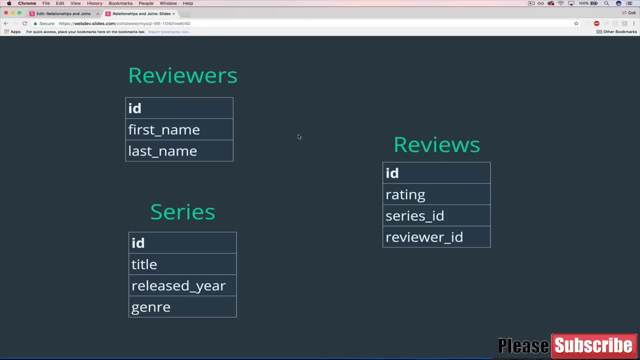 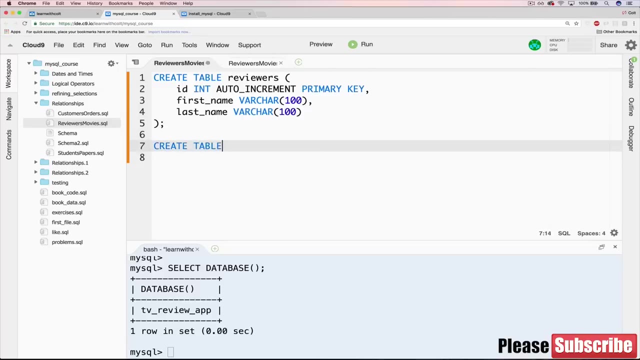 The next thing that we'll move on to: before we insert things, let's actually get our tables going. So all tables first, and then we'll insert our data. So next up we'll do Series: Title, Release Year and Genre. So Create Table Series And inside here we'll have 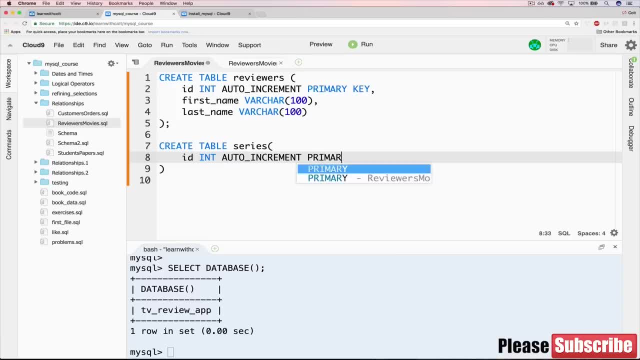 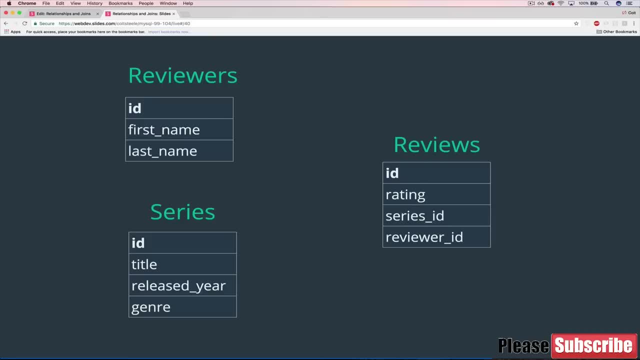 an ID which will be exactly the same Auto increment primary key. These primary keys are especially important because we're going to use them as foreign keys in the Reviews table and we need to have valid rows that we're pointing back to. So we need to make 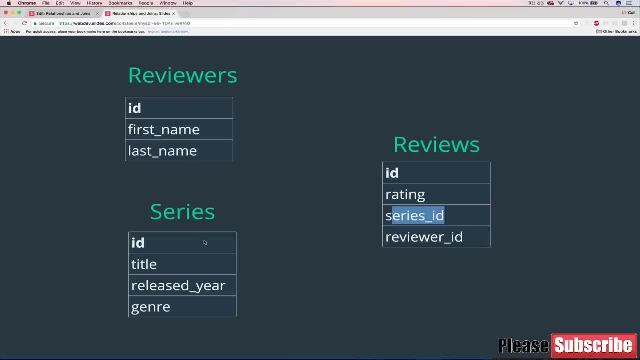 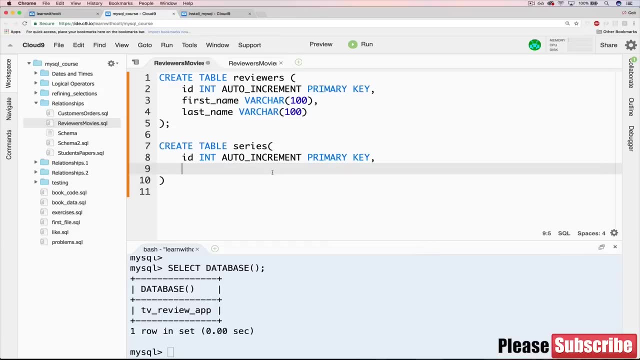 sure, whatever the series ID is here, that it's actually a series in our database, So it's not pointing to some non-existent show or non-existent reviewer in the case of reviewer ID. Okay, so the next thing is the title of the series, which we'll just make a varchar, And 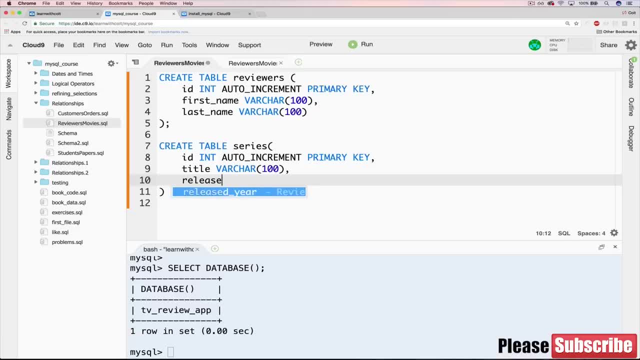 then, once we do that, we'll move on to Release Date, or Release Year in our case, And we have a couple of options for the data type here, So we could make it a date, but all we want is the year, And a date has this kind of format. 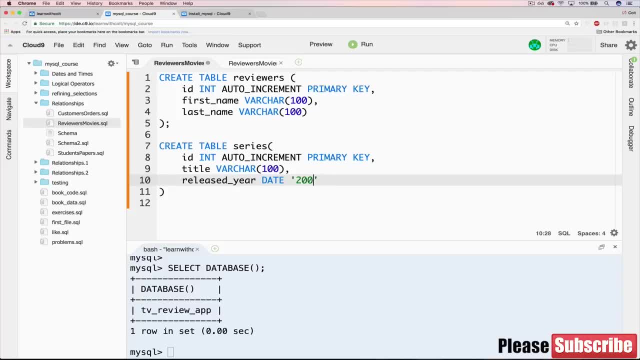 the year and then the months, and then you know and so on, which we don't care about. So we could make it an int And that would work. but then potentially someone could accidentally insert something with a release year of like 10,000 or 9999999, which is not a valid year. 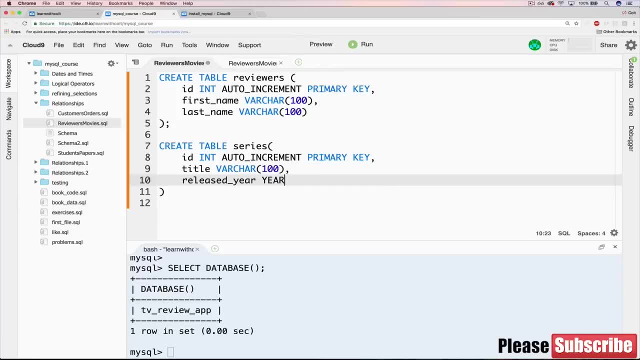 So there's actually another data type that we can work with, which I haven't shown you. It's just called year, And if we do year four, it will be a four-digit year, Like 1999 or 2004.. There used to be a year two type, but I believe it's been deprecated. 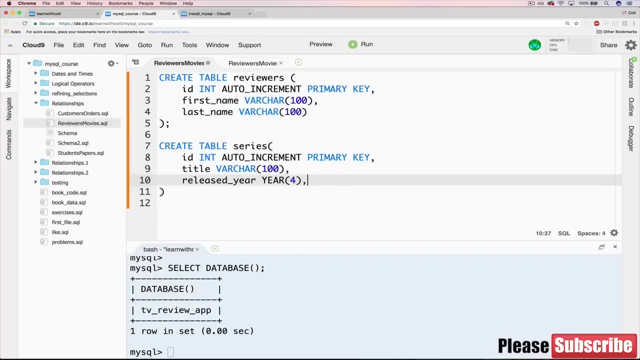 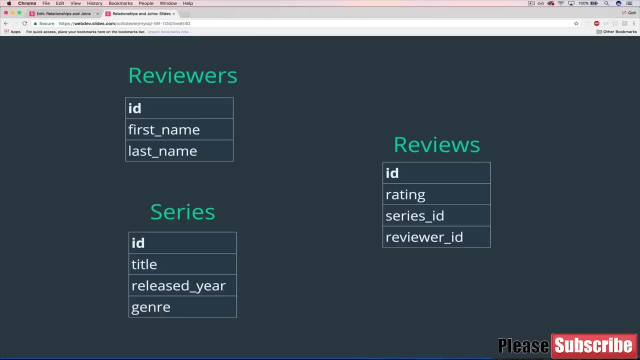 now, So we'll work with year four. That's not the point of this lecture, so don't let that hang you up. I just wanted to show you that it exists. So we have that, And then the next thing that we have is genre, And genre will just be a. 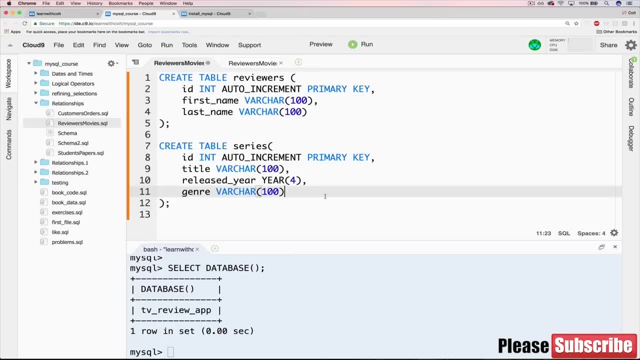 varchar as well. Okay, so we have those two tables. Now let's actually start with those and let's make sure that they work. So there's our first one And here's our second series. Great, Now, what I'm going to do is: 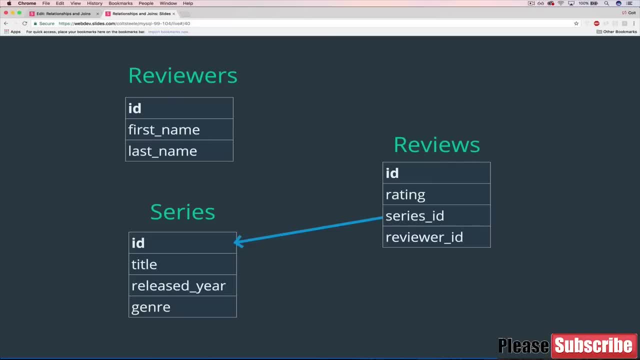 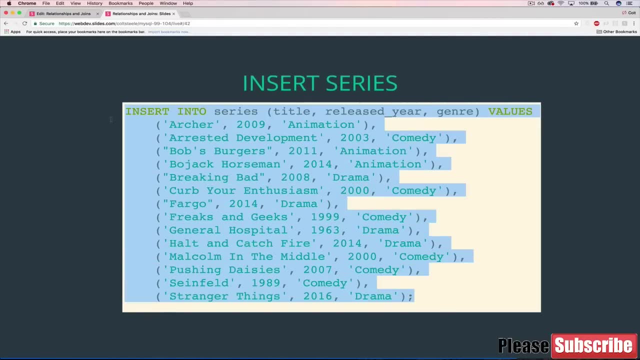 actually insert some data. We'll come back to reviews in a moment, So I have a bunch of series data here. You can, of course, copy and paste it from the included code, which is what I recommend you doing, because this took forever to type, Although. 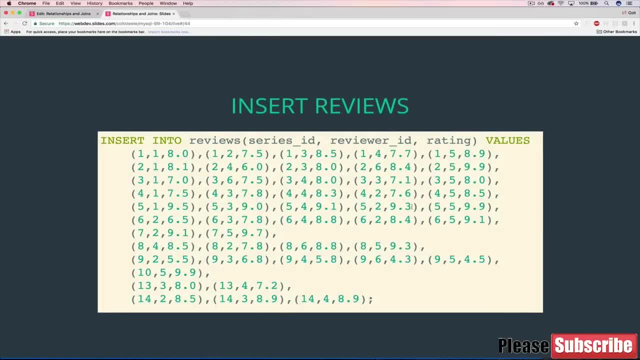 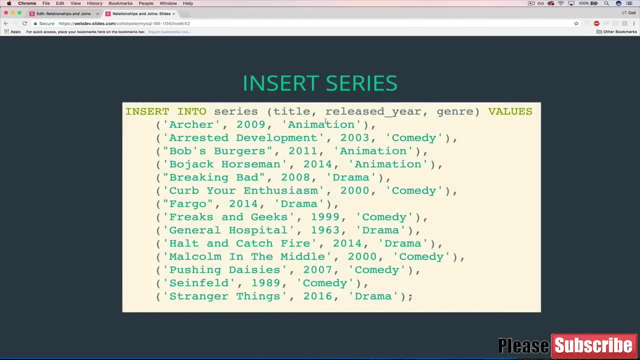 it's not as bad. I'll give you a preview of what our reviews data looks like. That was a pain to type, So this isn't as bad. But we've got shows. Most of them are shows that I picked because I liked them, But I also pick some because I didn't like them, so that we have some variation. 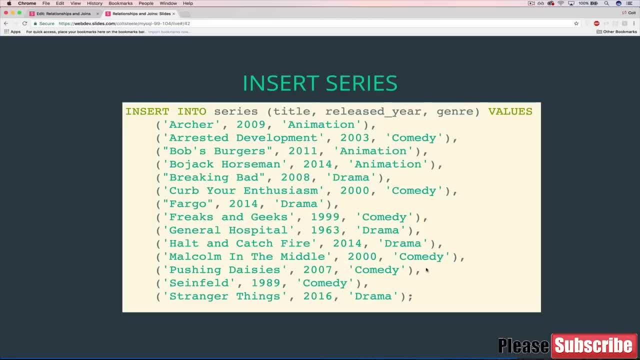 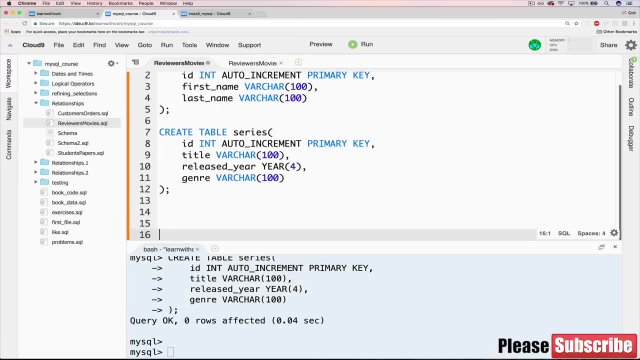 in the ratings. in particular, I want to make sure that our data was realistic and not everything was a 9.0. So I'm just going to copy this over, put it in this file, so we have a record of it and I'm going to. 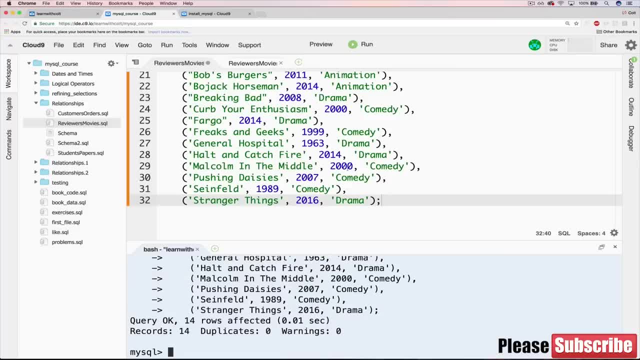 insert it, make sure it works. Okay. So that was 14 series we just inserted, And I'll do this one by doing run runue. Now an En Tulio column text appears And then that will be showing you the number. Hey, let's do. 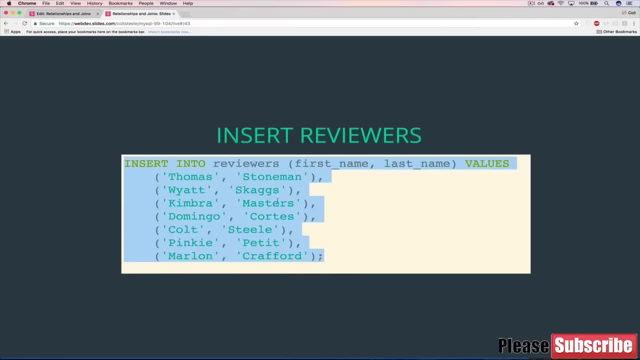 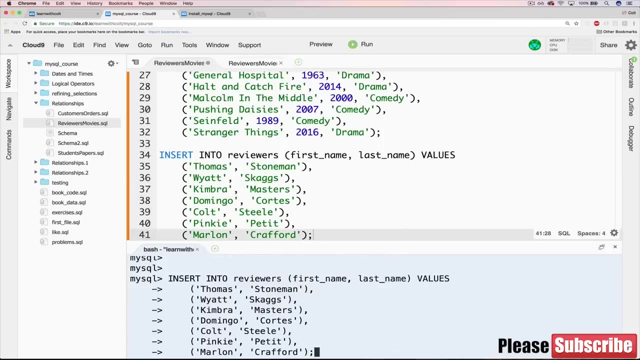 an En Tulio column text And this would style, depending on what we're someday using, or- And I'll do the same thing for reviewers. we only have seven here, but that's plenty And we'll paste it in Now. let's make sure it works. 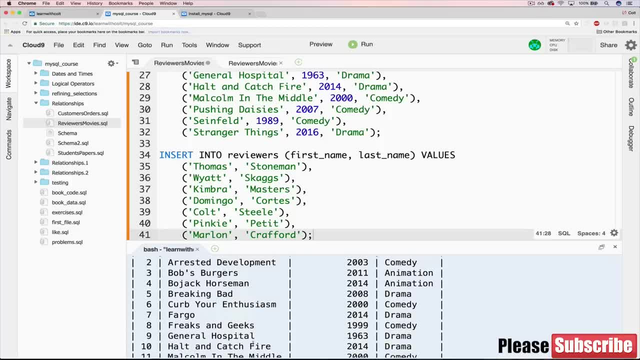 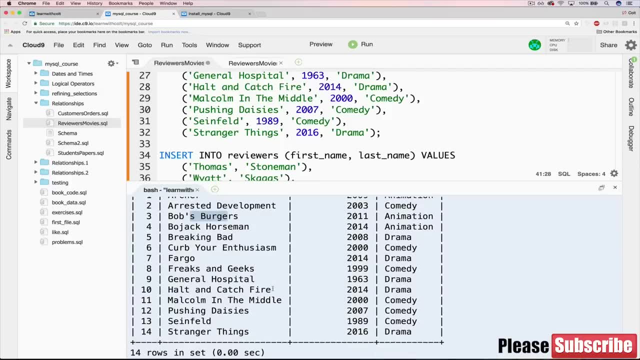 Let's do a select star from series to start. You can see, let me make this a bit bigger. here's all of our series: Archer, Arrested Development, Bob's Burgers, all the way down. we've got animation, comedy and dramas. 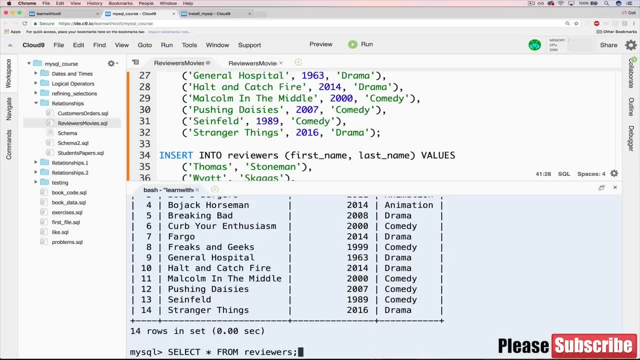 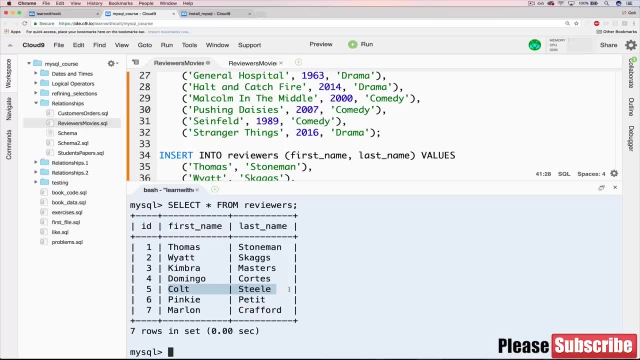 And then let's do a select star from reviewers And we've got seven of them, totally random names, except I did put myself in there purely so that I could review my own shows that I, like Everyone else has fictional- just totally made up reviews. but the ones that I put in 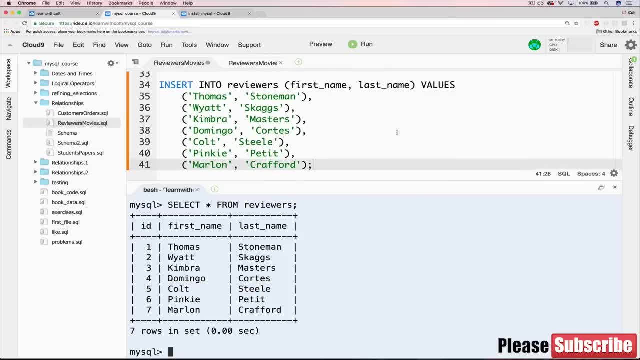 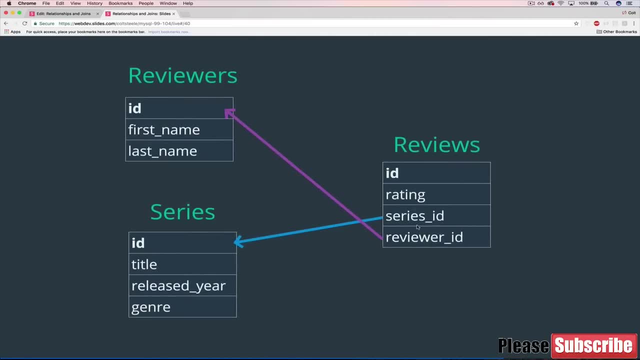 there are relatively accurate to my personal TV tastes. Okay, So then that leaves us with having to now implement the reviews table, which we left for last. For one thing, it depends on these two tables and it's also a little bit more complicated. 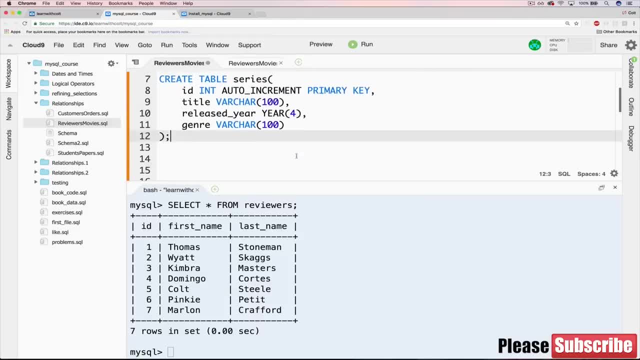 So let's get started. Scroll back up. I like to do all of our kind of schema code up top. So we'll create table and this is reviews, And the first part's easy or easy enough. We'll have an ID which is an int auto increment primary key. 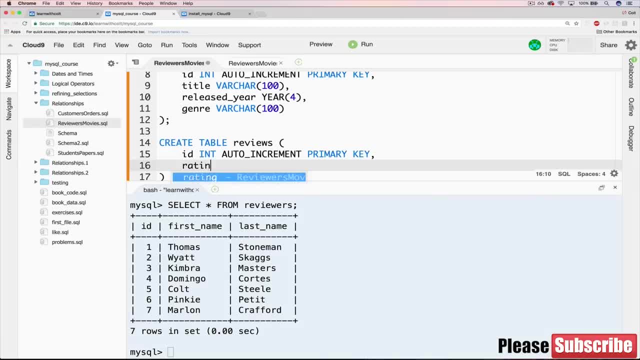 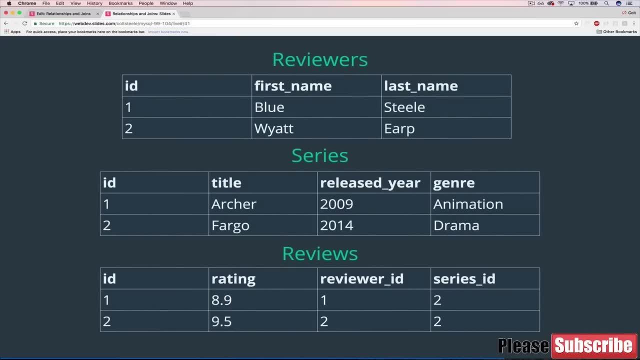 And then the next part's pretty simple too, which is rating. Now, what data type do we want rating to be? If we look at the examples I've given you, we have 8.9, 9.5.. So we could have just done an integer, and that would work. 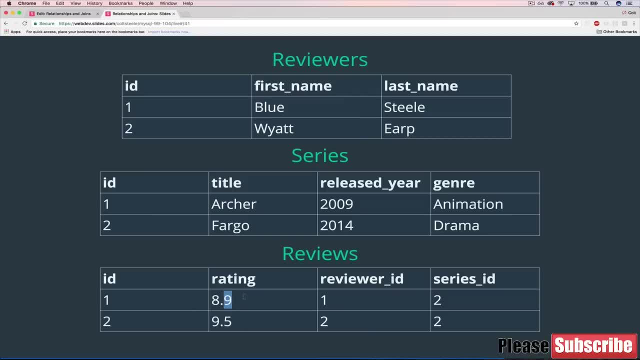 But that's not the way that we're going to go here, because we want decimals after it. So we could have just only allowed whole numbers from 1 to 10.. But instead we're going to do sort of like IMDB does, where they have a decimal system. 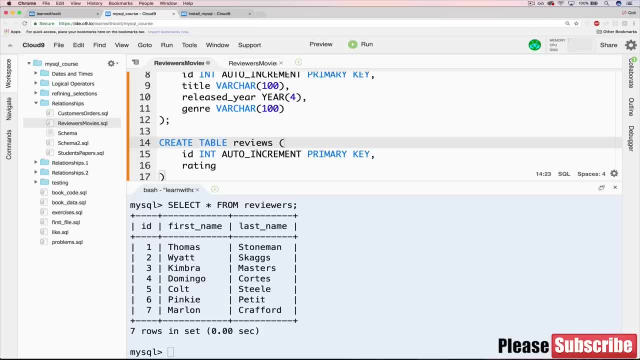 And our maximum rating will be 9.9.. So 0.9.. So that's going to be a decimal And if you think back to the section on data types, there are two things we pass into the decimal. The first is the total number of digits we want allowed, which is just 2.. 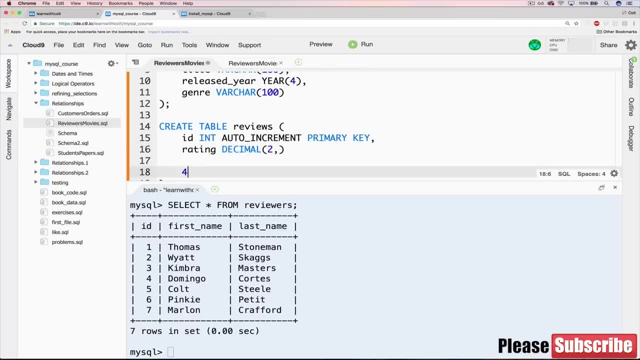 Because we only want things like 4.4. We don't want 43.4.. We don't want 99.9.. And then the second is: how many things or how many numbers after the decimal place? We just want 1.. 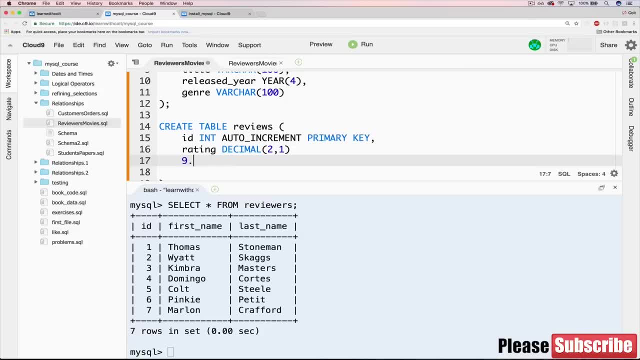 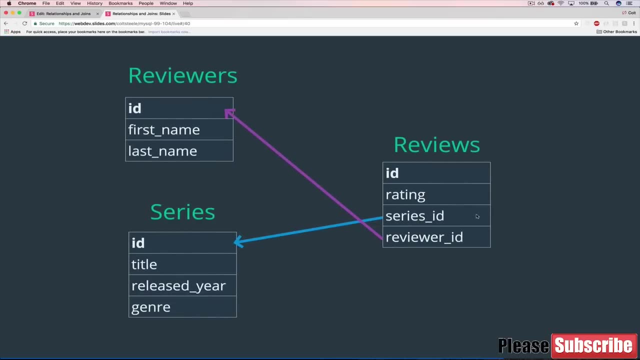 So that will give us two total numbers like 9.9 or 5.6, something like that. So that's all we need there. Now we get to, if we go back: series ID and reviewer ID, So both of those will just be integers. 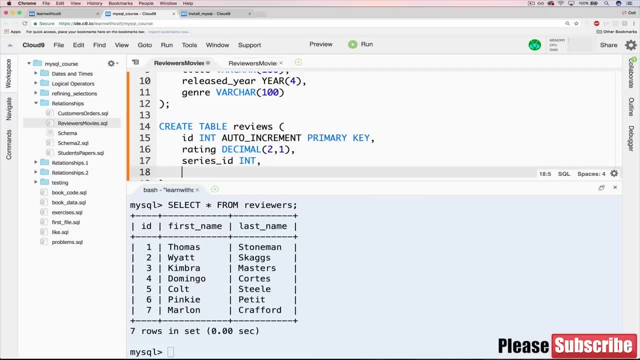 So we'll just start with that Series ID is an int And reviewer ID is an int as well, But of course we're not done, We're not done yet, We're not done yet, We're not done, yet that they are foreign keys. 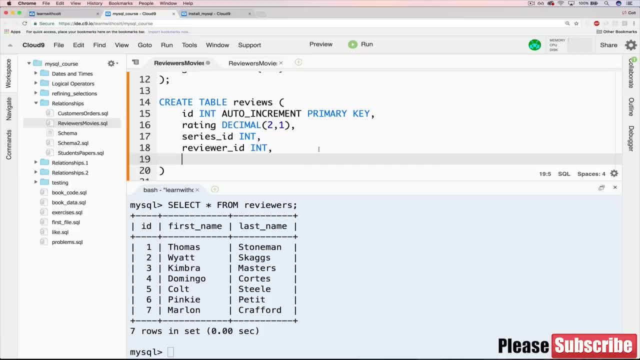 Remember from the last section. you don't have to do that, but it's a really smart thing to do to enforce that when you insert a review it actually corresponds to a valid series and valid review. So the syntax for this it's been a little bit. 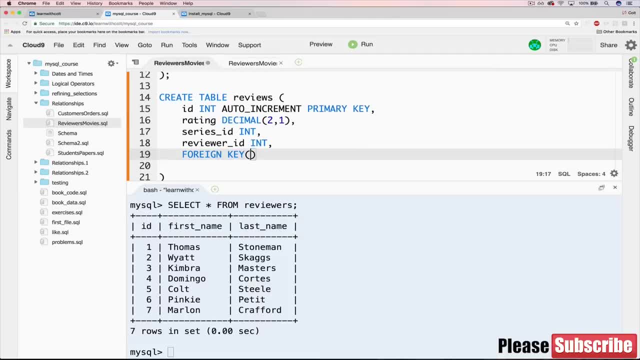 but it's foreign key and then we tell it we'll work with a series ID first. So we're saying, okay, this field series ID is a foreign key. references and what is it referencing: The series table and what field. 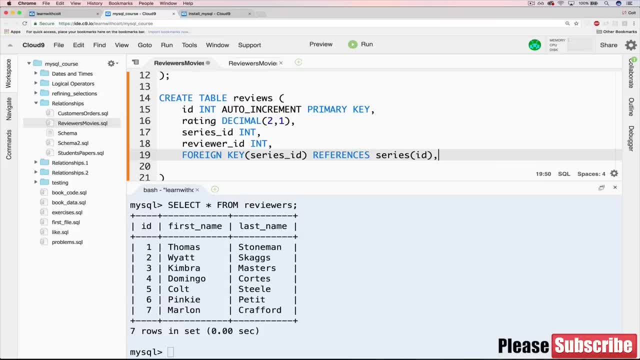 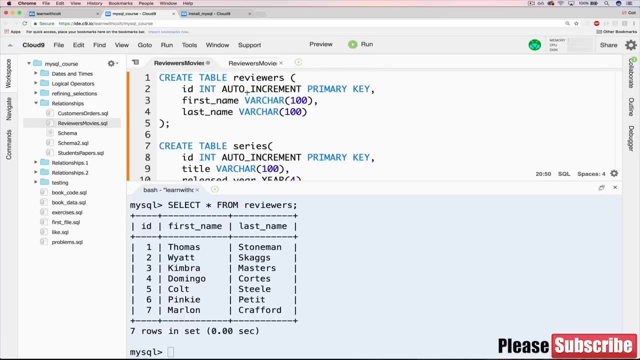 The ID field. so just like that. And then we'll do the same thing, but this time we're saying this reviewer ID field, right here is a foreign key references the reviewer. table up here the ID field there. Oops, there we go. 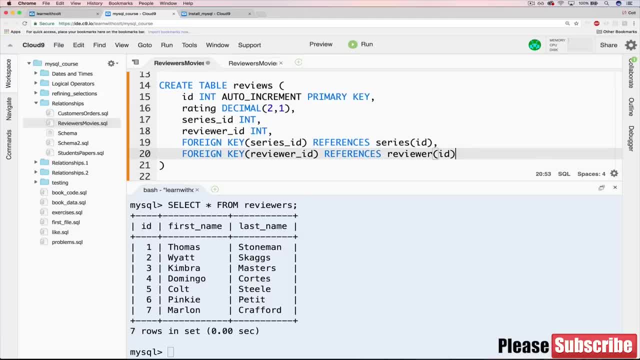 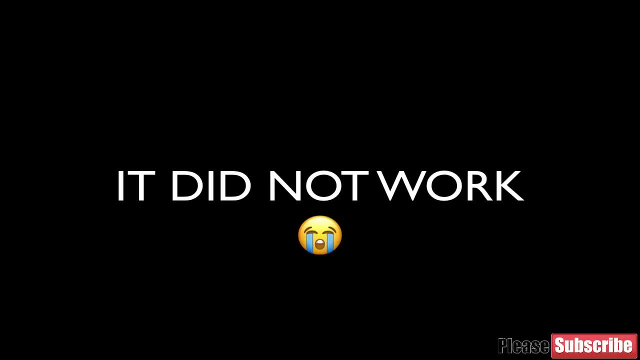 Let's make sure we have commas in the right places, add in our semicolon at the end and let's see if it works. So there is a mistake in this code. I've already gone back and edited this, but I kept this in here because it's a mistake. 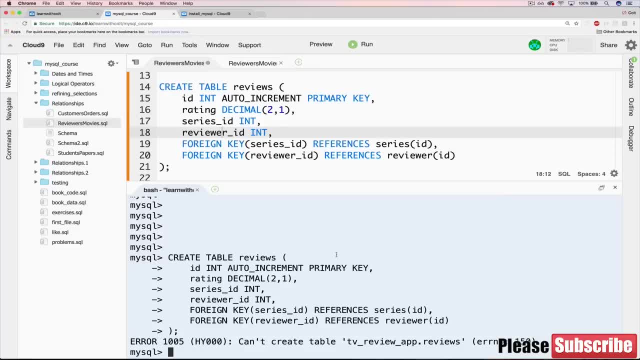 that I think is pretty common and it's a little tough to spot. If you look at, maybe you already spotted it, but if you look at the error I get, it says can't create table. it's really not very useful. 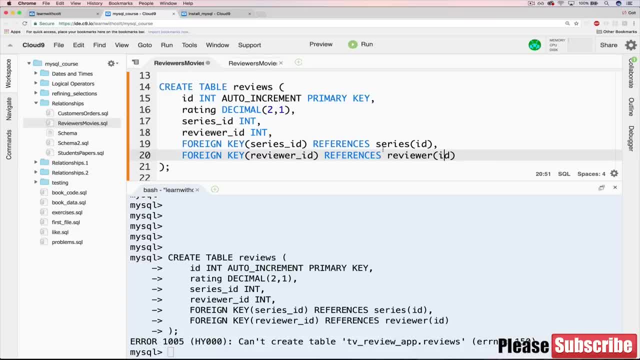 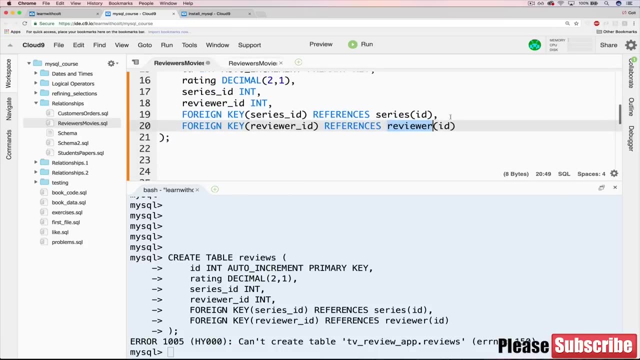 But what's happening here? typically, if we get an error like that, it has something to do with foreign keys here. and the main thing, remember that these are referencing external tables. so we have a series table, but we don't have a reviewer singular table. it's reviewers. 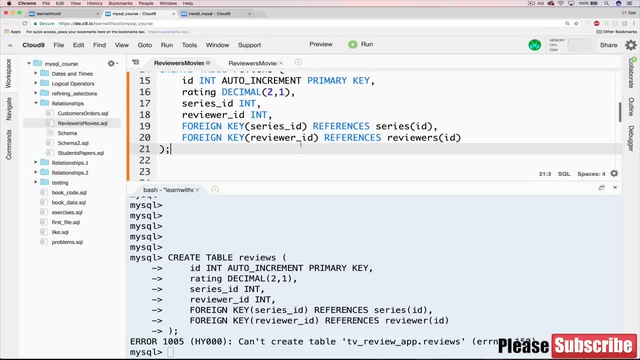 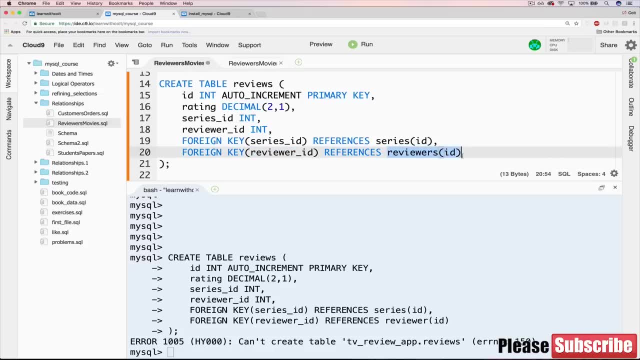 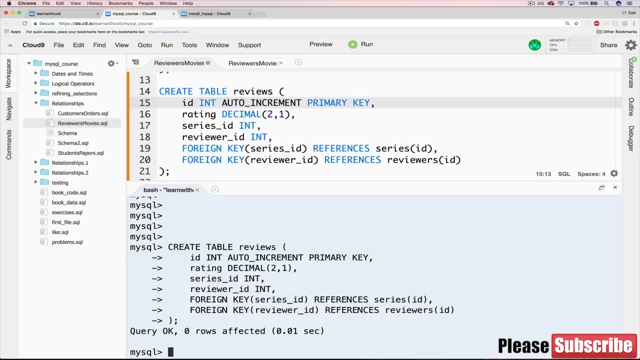 So I end up doing that quite often. I see some of my students do that often as well, because sometimes you just talk about things in singular. we have reviewer ID versus reviewers ID here. it's very easy to mess that up Now. hopefully it should work just fine. 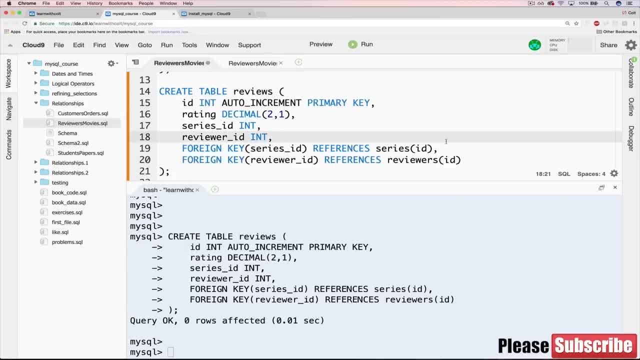 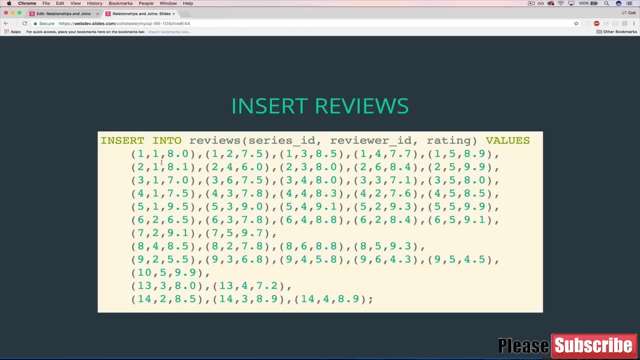 and it appears to Okay, so we still don't have any data in there. the last thing that we'll do is copy and paste this monster, all these reviews- this was like an hour- to try and get this with some realistic data. 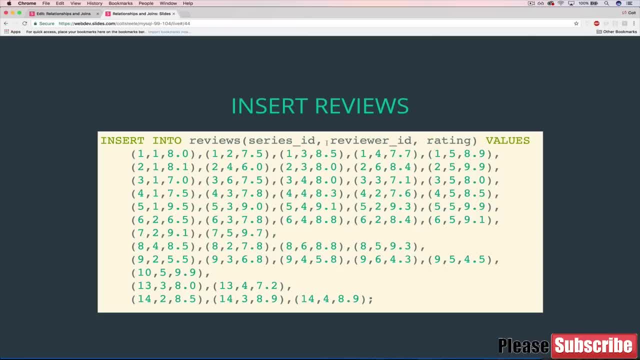 So I wanted numbers that accurately- relatively accurately- reflected the quality of shows. Now, you may disagree with it, but copy this in. definitely don't waste time. don't waste time typing this yourself. Copy it from the code that I've provided and paste it. 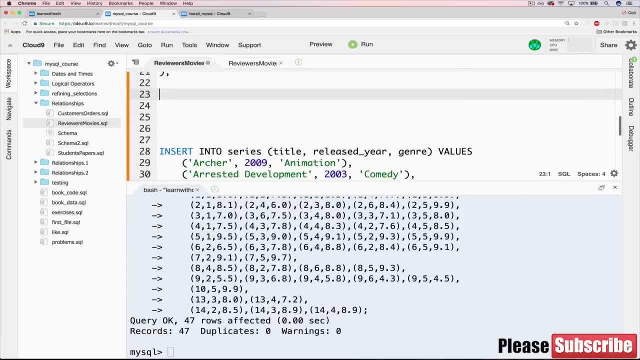 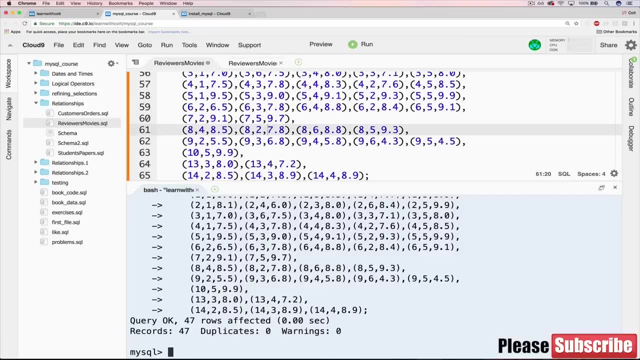 Okay, so now we should be good to go. I'm just going to add this in here so we have a record of it And just to double check that everything worked. we're just gonna select star from reviews and we'll leave it at that. 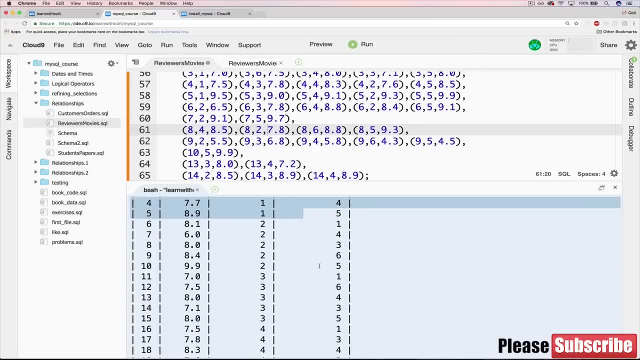 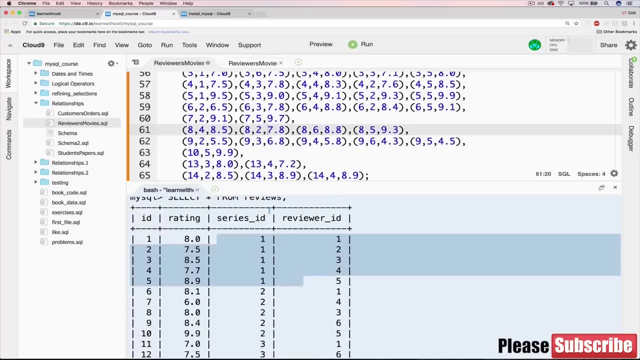 So, as long as we see our data in here, notice how difficult it is to understand. What does any of this really mean? At the moment, nothing, unless you happen to know you have memorized the different IDs for series and for reviewers. 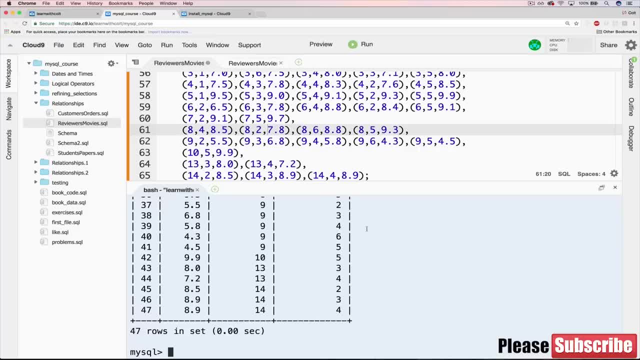 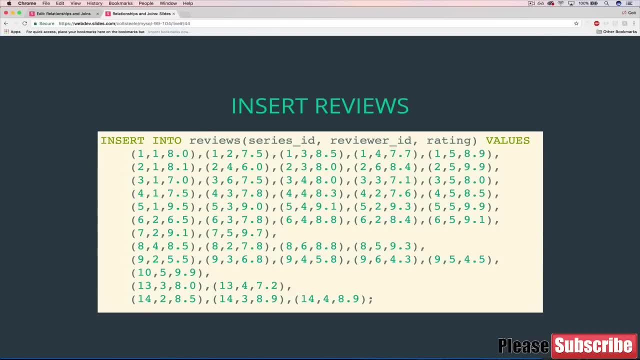 So that was preparing our data, creating our schema and inserting our sample data. Next up, we're gonna start working with it. All right, so we inserted all of our data. we have our schema ready and all of our tables created. 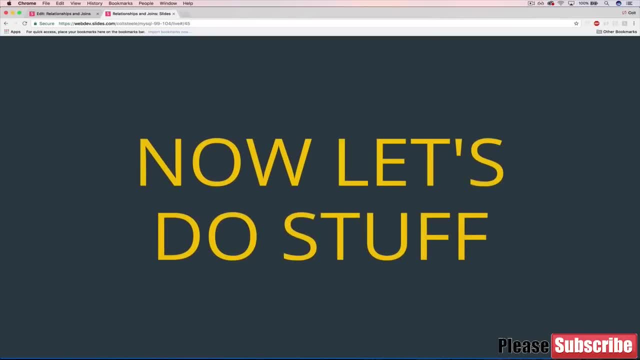 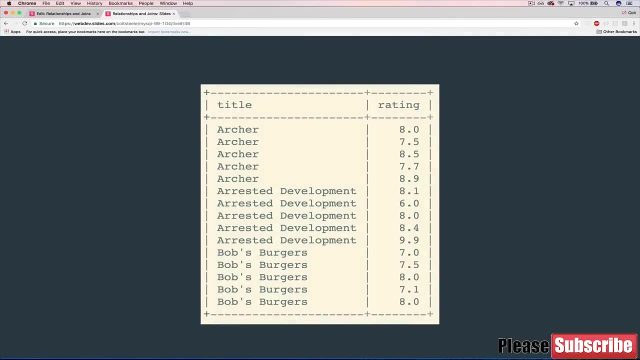 Now let's get down to business. Let's do some stuff with it. So I'm gonna break every problem that I'm gonna give you- and there's quite a few here- into its own video. Hopefully it'll make them a bit more manageable. 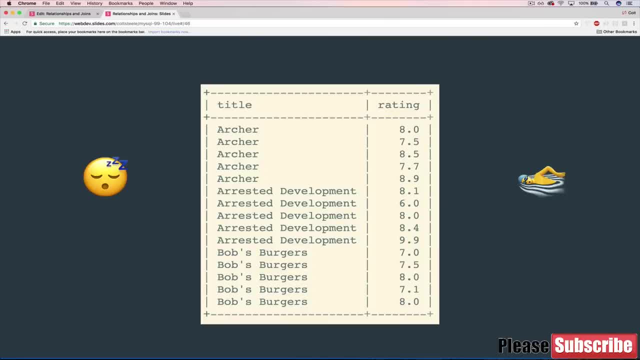 and you won't wanna go to sleep or drown yourself after watching it. So the first thing that you'll see here- the format of these- is that I'm gonna give you the results. It's much easier just to give you a picture of them. 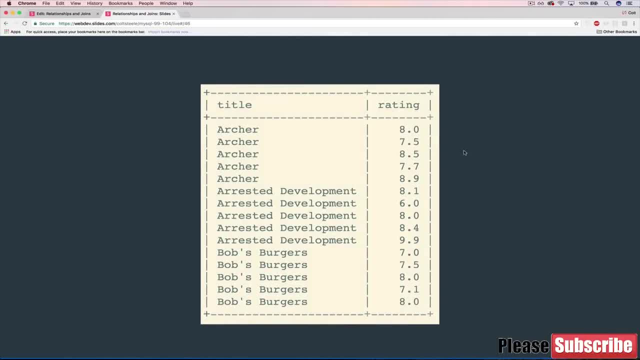 rather than trying to describe in a bunch of text what it actually means, It's much easier just to show you. So first thing I should say is that these results are truncated. These are only for the first 15 or so. I used limit, but I want results for everything. 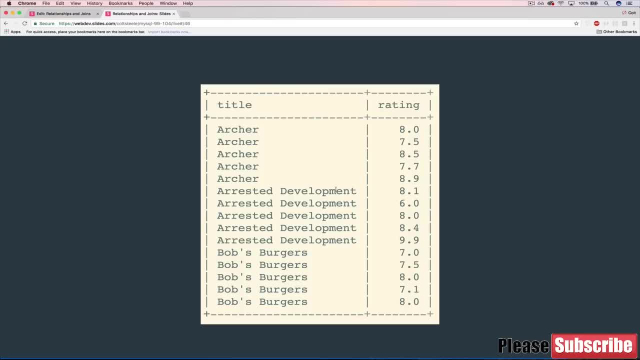 It's just too hard to fit them onto the screen. They'd be very, very tiny. But the key thing is that we have title for a movie or, excuse me, for a series and a corresponding rating. So we're going to need to join those tables together. 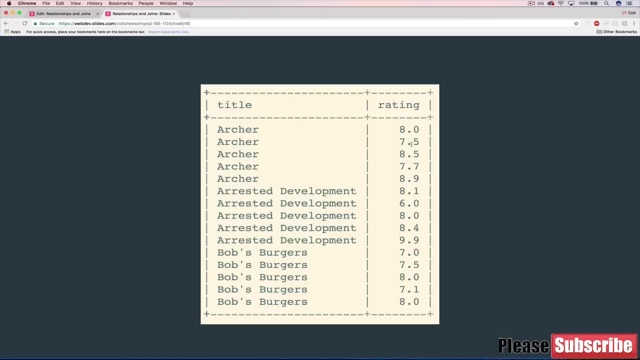 We need to join the series table with the reviews table, because right now they're not in the same table. We're storing the titles separately from the ratings, So let's do this now. We'll go over to Cloudflare. We'll go over to Cloudflare. 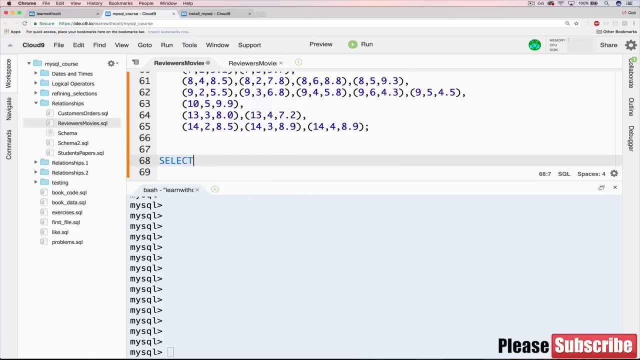 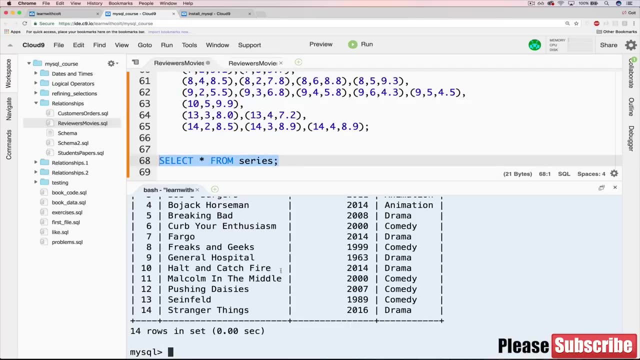 We'll go over to Cloudflare, We'll go over to Cloud9.. And the first thing we'll do is just start simple. We'll select star And we'll just start from series, which we've already done, Just like this. 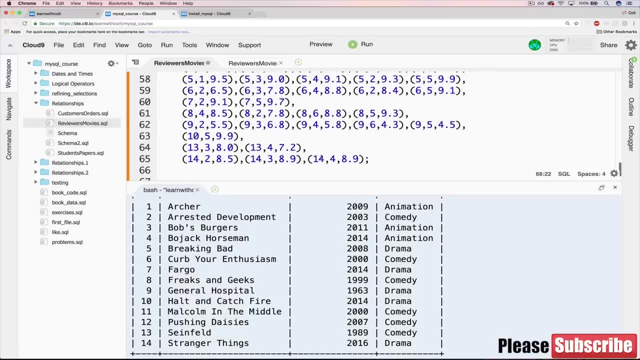 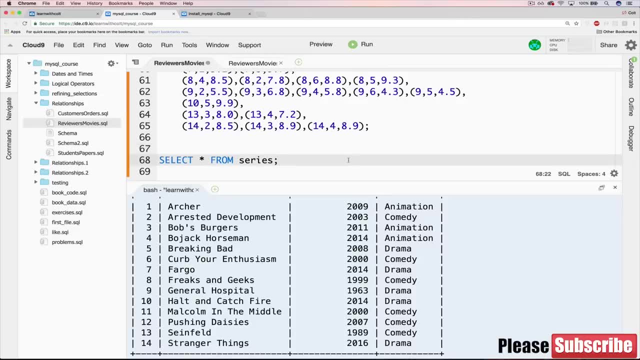 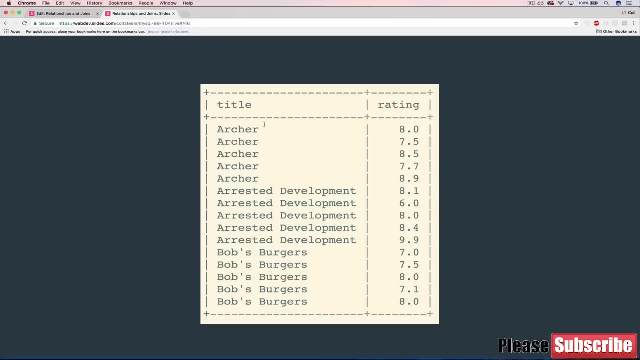 One thing I should highlight before we go too far. I did deliberately add some series that don't have any reviews so that nobody has rated them yet, And that was deliberate so that we can work with that later. However, in this example, I only want to see movies. I keep saying that. 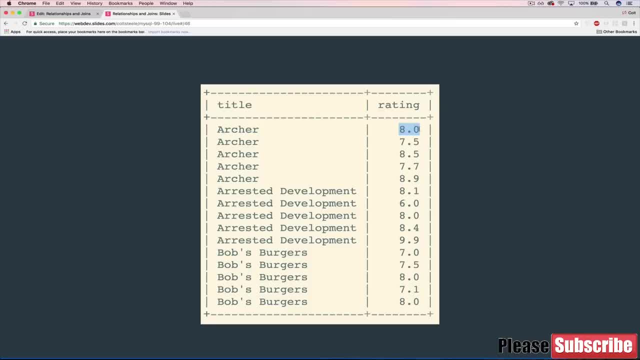 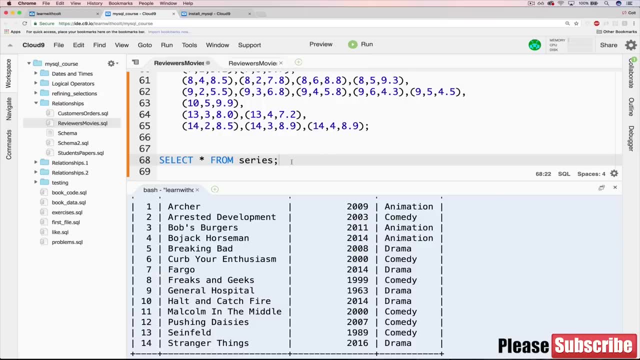 I only want to see titles of series that have been rated, So we don't have any nulls in here, which is a bit of a hint. So select star from series and on its own, we get this. Now, what we want to do is join. 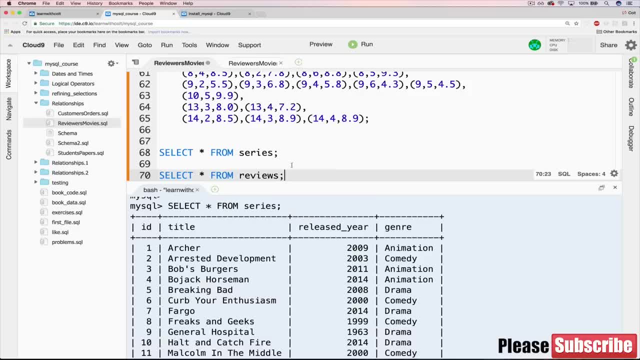 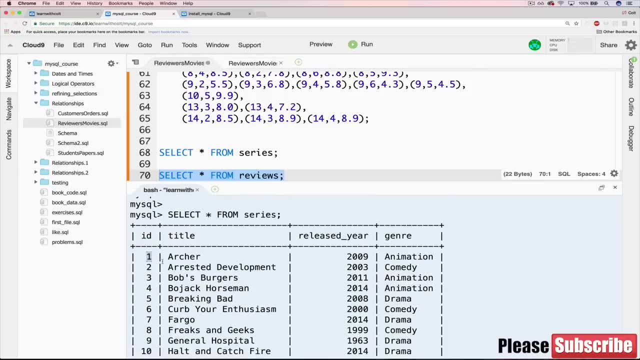 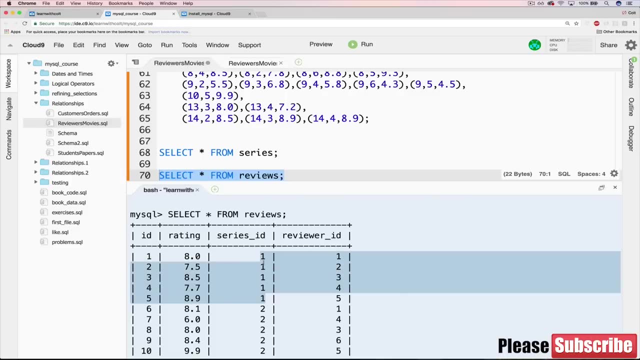 So if we do a separate select star from reviews, we want to join basically where this ID of the series is the same as the series ID. So these first. let's see five here: one, two, three, four, five. 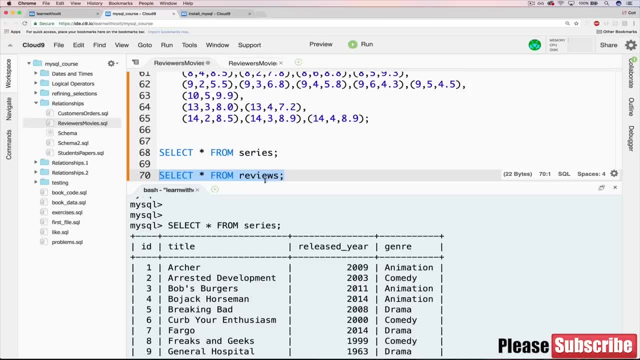 correspond to archer, which is what we see here. So to do that we don't need two separate selects. We want to do select star from series. We'll do join with reviews On, On, On. And where do we want? 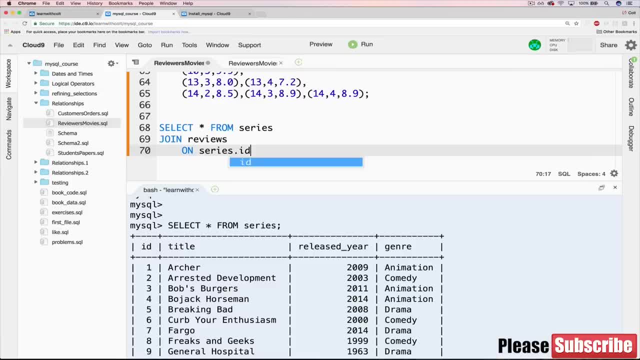 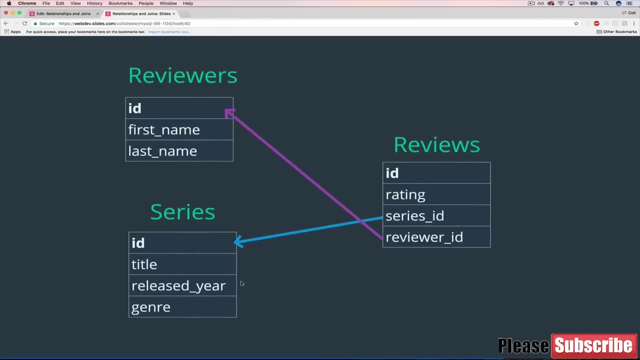 We want to join on seriesid equal to reviewsseries underscore ID. Just to reiterate where this ID of the series actually it's going to be easier if I do it here- Where this series ID is equal to this ID of the series table. 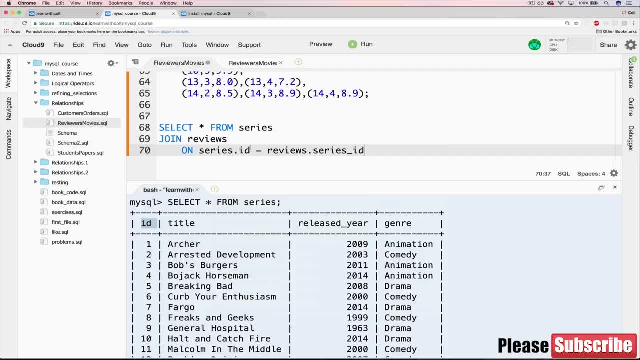 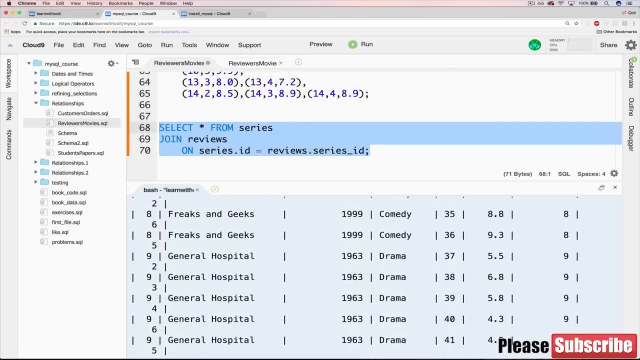 Okay, And all we want are title and ratings. But we'll start with just getting everything and let's see if we're in business yet. Well, it's a little hard to tell because we have this formatting issue where we have so much data. things are being cascaded over. 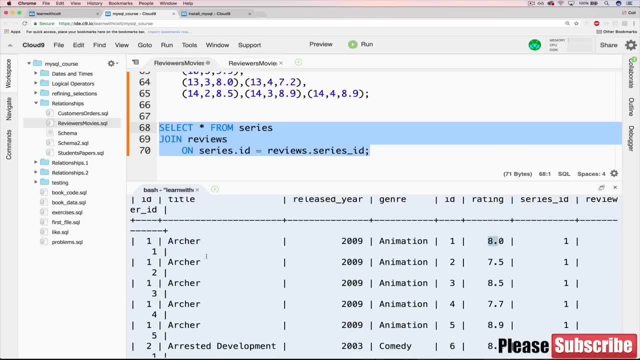 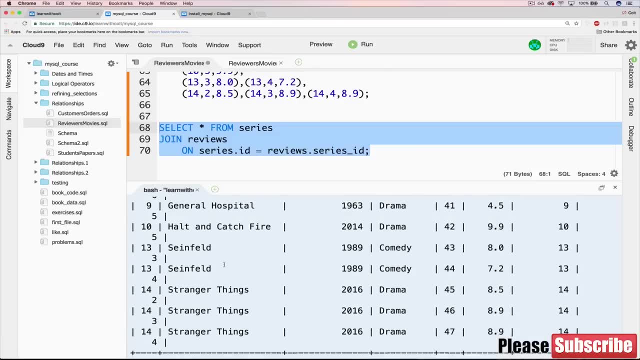 But if we look closely we can see, okay, we have Archer 8.0,, Archer 7.5, Archer 8.5, and so on, And if we scroll down you can see that not every single TV show is here. 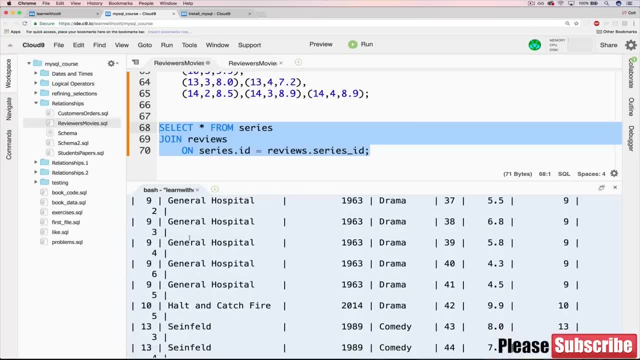 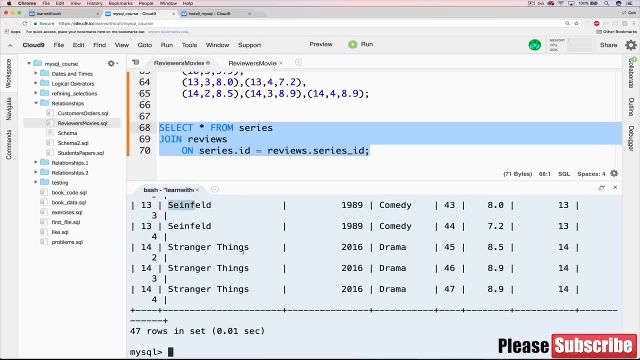 I think you'll notice the IDs jump 7,, 8,, 9,, General Hospital, 10,, Halt and Catch Fire then goes up to 13.. So, whatever 11 and 12 are, we don't have any reviews. 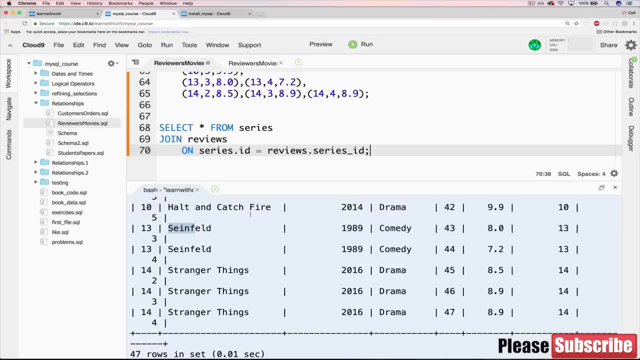 So that's good. Not that we don't have reviews, That's not good, But they're not showing up, which is what we want. So now we'll just whittle this down to title and rating, And that's all we want. 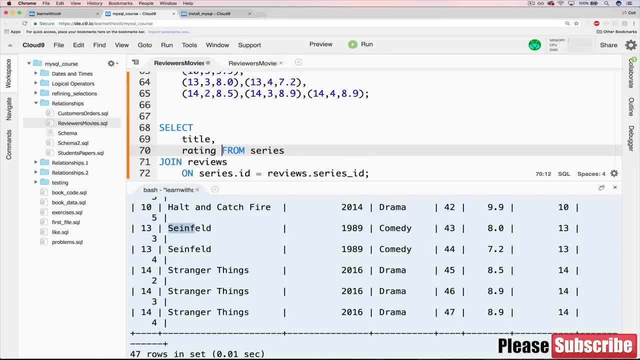 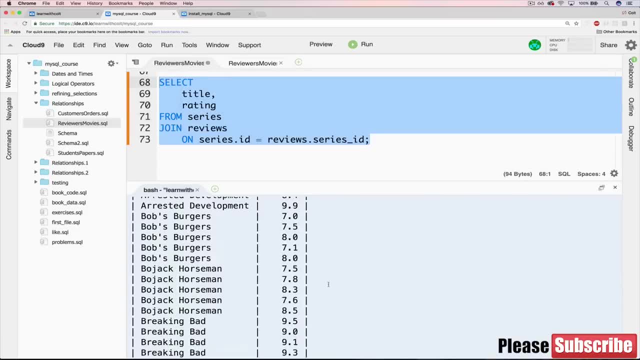 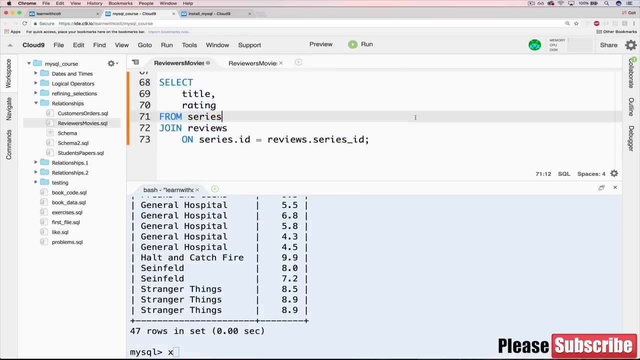 And I'll format it a little bit nicer. Here we go, Hit enter And now, And now we get all of our data. On the left side we have title. On the right side we have corresponding ratings. So hopefully what we just did there seemed relatively similar to what we did in the last. 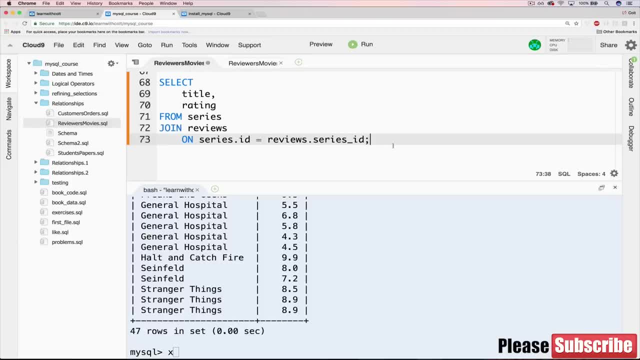 section where we were writing these joins. What we'll build up to in this section is doing a double join where we have another join statement because we want to connect all three of our tables. But for now we're working with one table or two tables at a time. 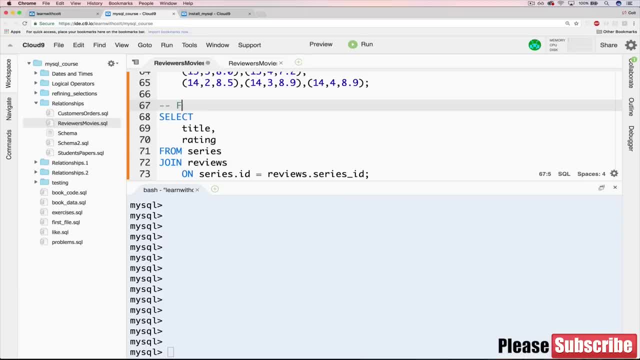 Okay, so we're done with that one. Let me just put a comment up here First. let me just do challenge one And now we'll move on. Next video we'll pick up with challenge two. Okay, moving on to our next little challenge here. 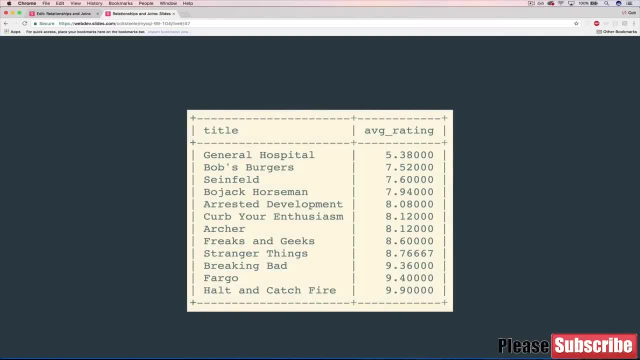 So here's what the end result should look like. We have two fields, just like we did in the previous one, But there's quite a bit of difference. If you notice, we have title still, so that's the same, But we only have one entry per series. 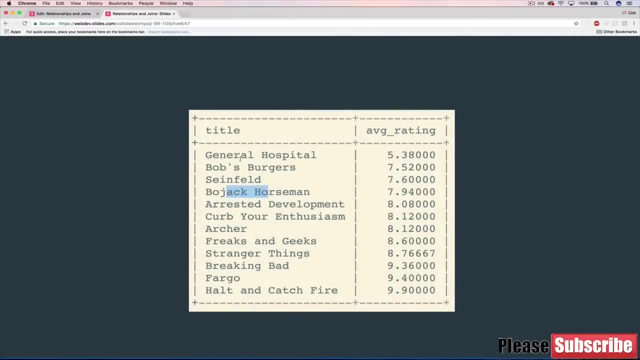 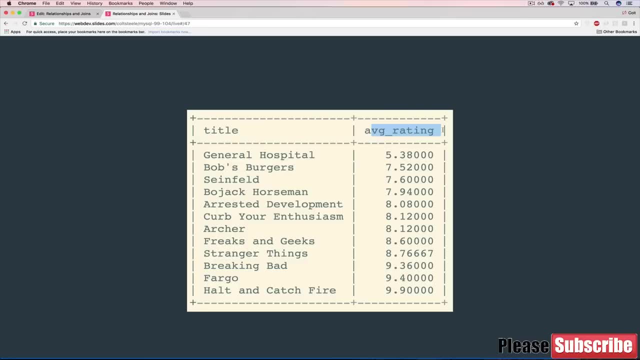 So we don't have, you know, Archer Archer, Archer, Archer, Archer. We just have Archer Archer, Archer, Archer, Archer, once somewhere. where are you Over here? But we also have average rating. So this is for all of the reviews, all the ratings for a given title. 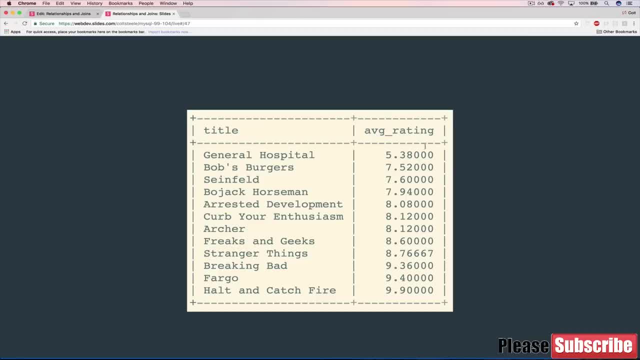 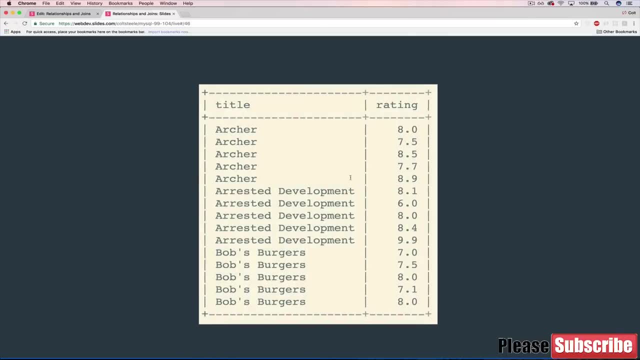 Put them all together and find the average. And then the other thing is that the results are then ordered from lowest average to highest. So basically, we're going to work with very similar data and take a same approach, join the same two tables. 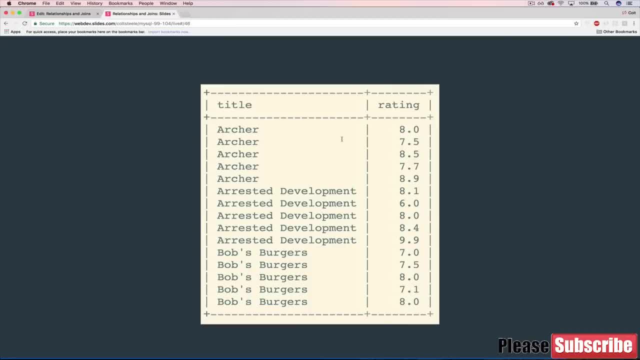 We're joining series with reviews, But then we're going to work with the same tables, But then we're going to work with the same tables to group them together, and then we're going to average the rating and then we're going to order. 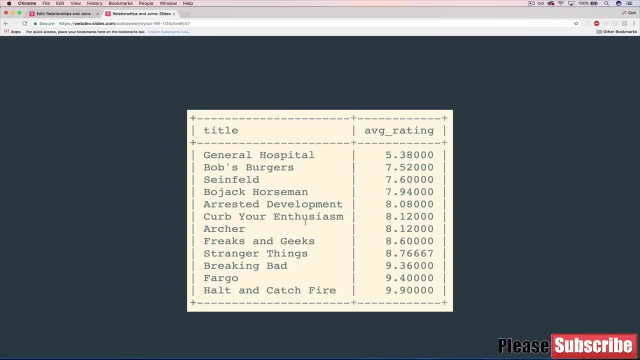 by average rating And, just like the previous problem, there are certain series that don't have reviews. They are not showing up here, So we don't need to worry about that. If we're worrying about nulls or non-existent data, that's not a problem for this particular challenge. 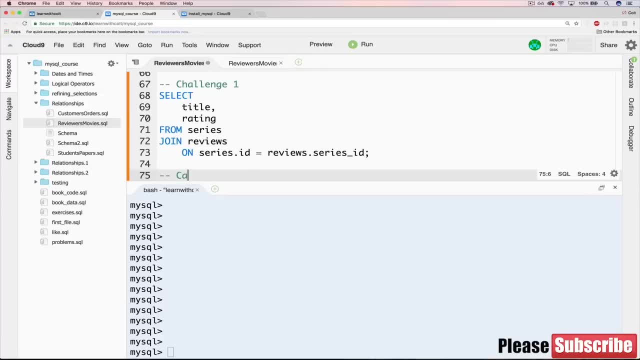 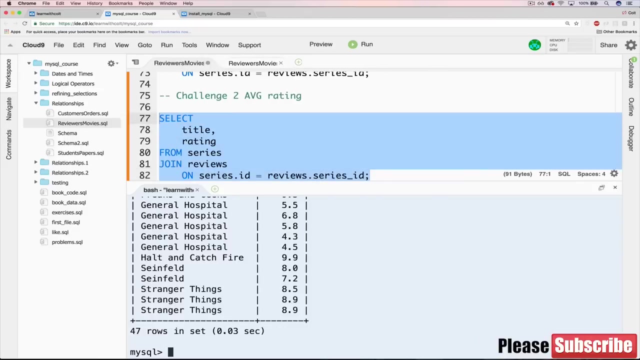 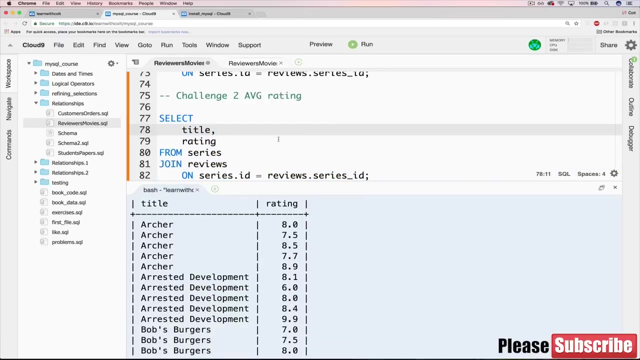 So we're going to call this challenge to average rating. So if we just actually type a very similar thing- so select title and rating from series join, reviews on seriesid equals reviewsseriesid- This is going to get us really close. We have all the data we need right here. This is it. We don't need IDs or we don't need. 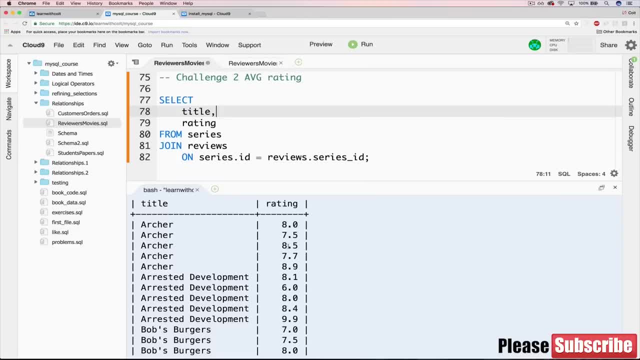 to worry about release years or genres or anything. This is all we need. However, we need to group things together so that all Archer reviews are together, all Arrested Development reviews are together, and so on. So then, that begs the question: how do we? 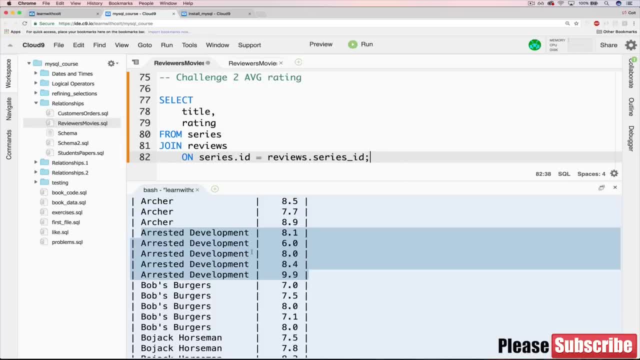 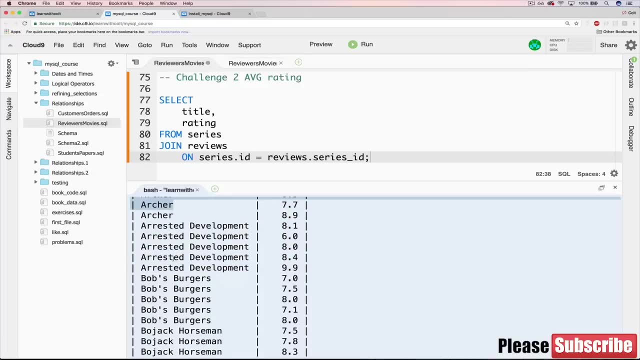 group them What's the best way, And there's a couple of approaches that we're going to use. Really, we could do it based off of the name, the title, But that assumes that there's only one show named Archer, one show named Bob's Burgers, which is probably true 99.9% of the time, But it's 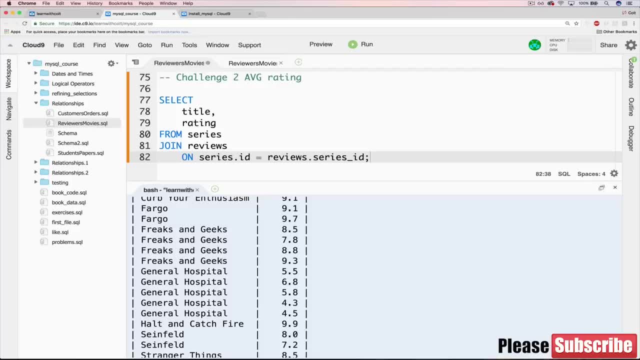 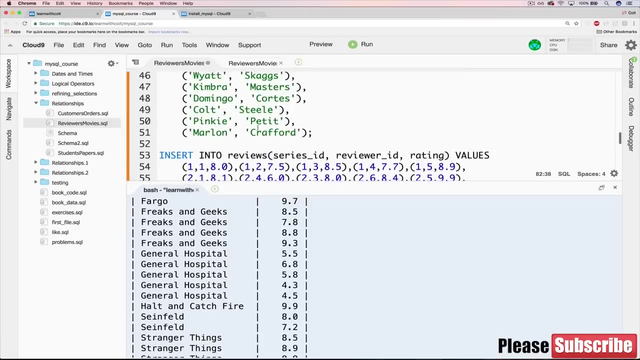 possible that we have shows with the same name, Or maybe there's a remake of a show I'm trying to think of- I know there's been examples of this- whether it's an older show that's been remade more recently. But basically it's best to not have to worry about that Because we're not making. 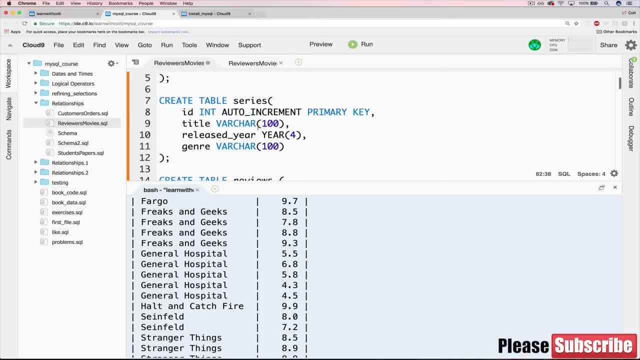 we're not enforcing that the name of the show is unique. If we go to series, the only thing that has to be unique is ID. So it's much better to group based off of that ID. And of course it's here. Well, we're not seeing it printed out, But we can easily see it if 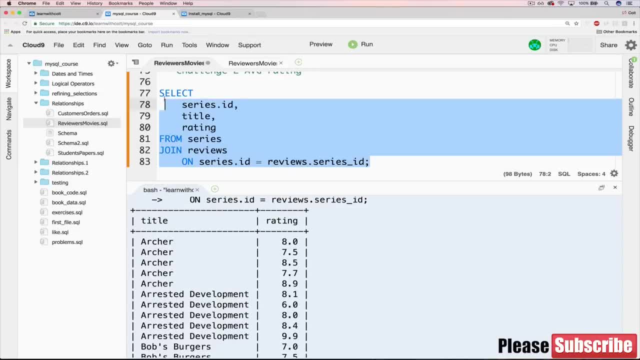 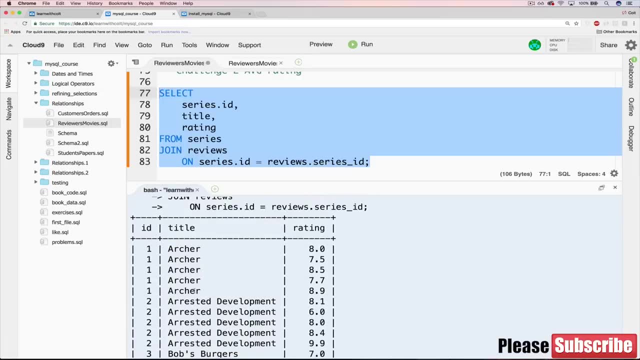 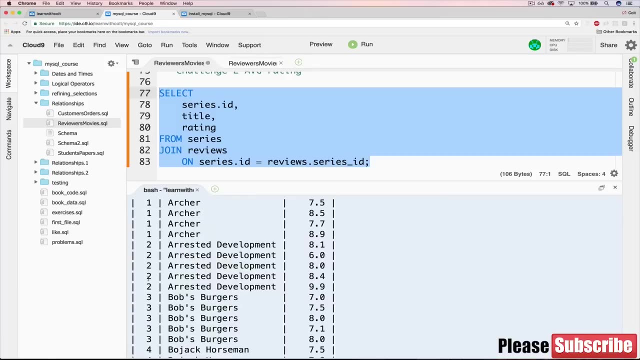 we just add in seriesid. So now if we run this you can see we have that ID there. So even if we had another show named Archer down at the bottom, we wouldn't have to worry about that. But if we go to the bottom with ID of 15, if we group by the series ID, then they'll be. 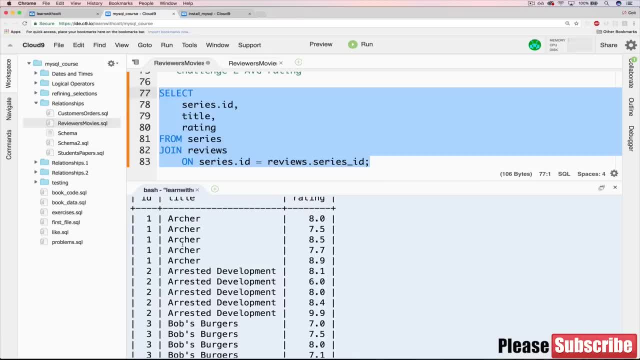 unique And they won't, you know, muddy the averages, they won't muddy the group by. So that should work fine And we don't actually need that series ID anymore. But we're going to do a group by And we need to do seriesid. That's important. If we just do ID, that is confusing Because it 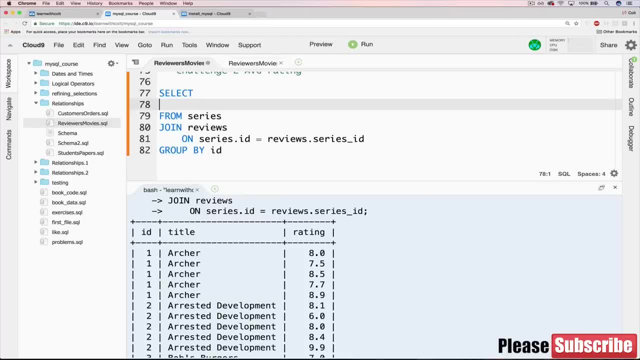 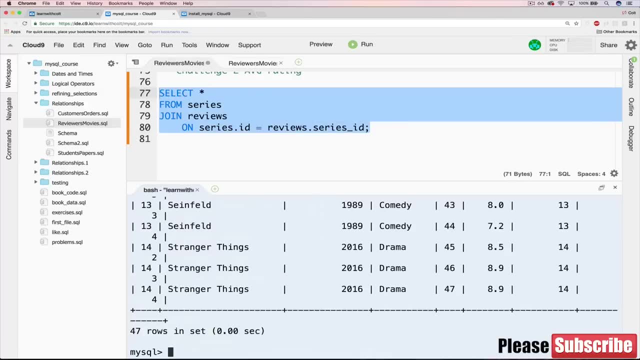 could also be reviewsid. Just to showcase that if we just select star- and I'll get rid of the group by- if we just select star, you can see, even though it's still messy, we've got one ID here. we've. 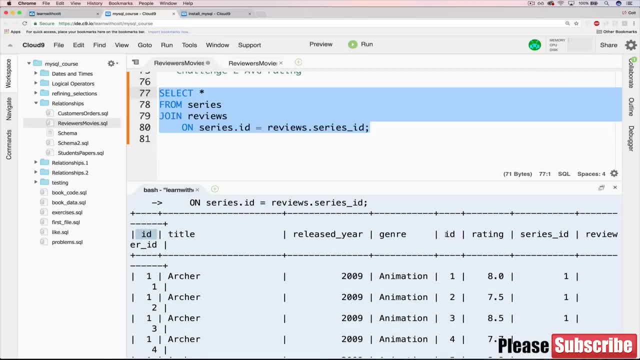 got another ID here. So this is the series ID And this here is the reviews ID. So we need to be explicit. Okay, so let's undo our changes, go back to what we had. we're going to group by seriesid. 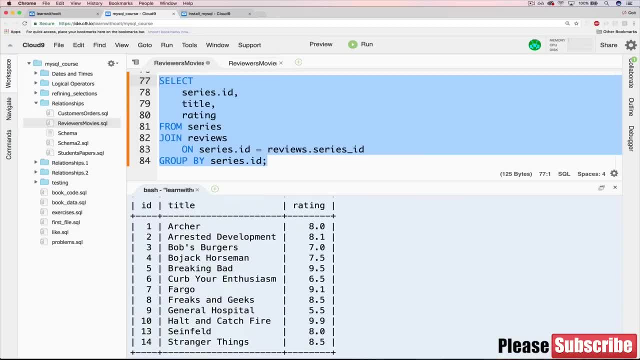 And if we just do that, it doesn't get us that far. It gets us closer, But rating is just going to be the basically the first one. Luckily, the draw essentially it's not an average, it's just showing us one rating. even though they're grouped by this ID here, we're still not getting the. 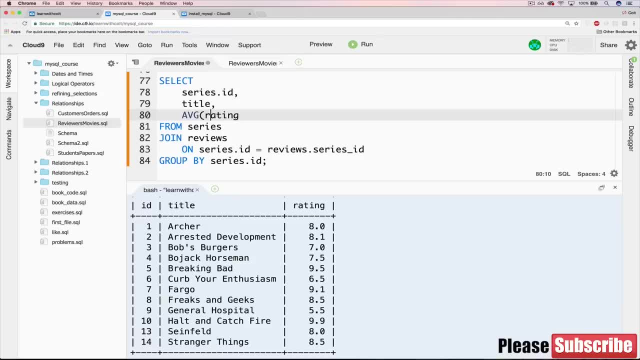 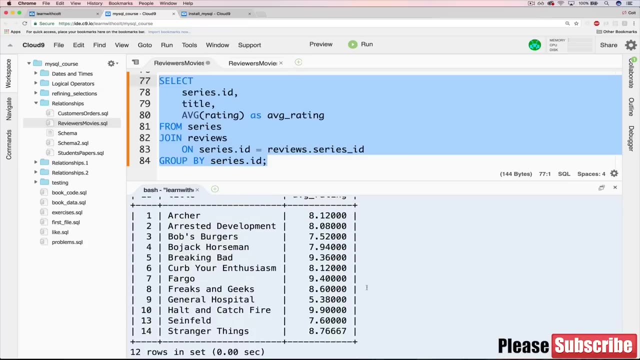 average, And that's a very simple thing to change. We just need to do average here, which we should be comfortable with by now, And let's give it an alias average rating, Just like that. Okay, let's take a look. Looking good, We've got title and average rating- a couple. 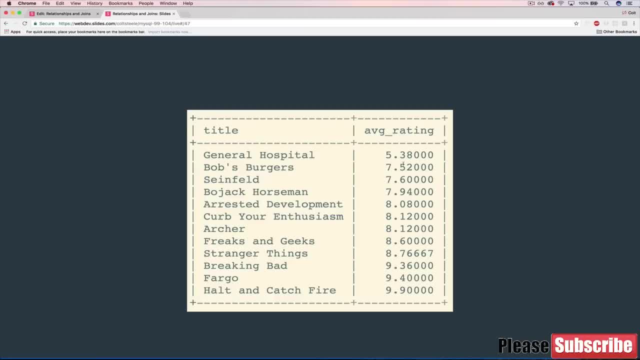 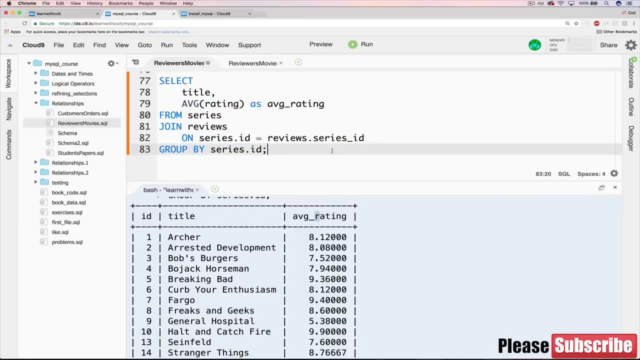 things: One, we need to get rid of ID, And two, we need to change the order. So let's start with a simple one: get rid of the ID. Then let's go ahead and at the end add an order by: So how do we want? 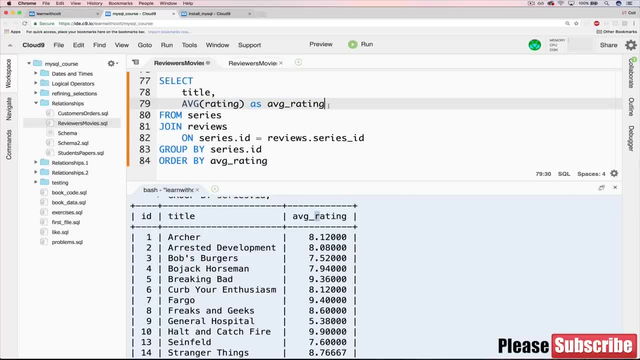 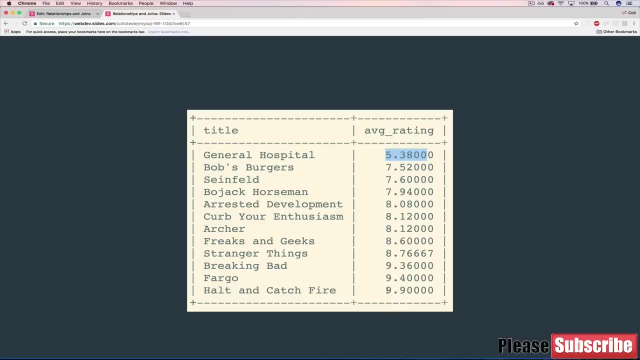 to order them. Well, what about just using average rating? So, order by average rating. and then, what order do we want? We can work with the default ascending order, Because that's what I have here, from 5.38 up to 9.9.. And there we go: 5.38 up to 9.9.. 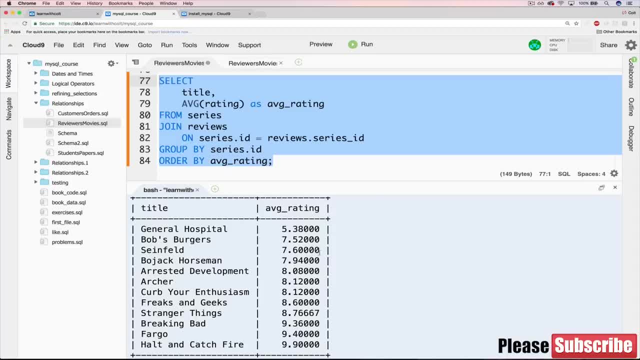 Now, that's basically the end, But I do want to highlight that these reviews are a little bit accurate. in my opinion at least General Hospital- not my favorite show- Only gets 5.3 on average. probably well deserved, I'm sorry, but I'm not sure, So let's go ahead and add an. 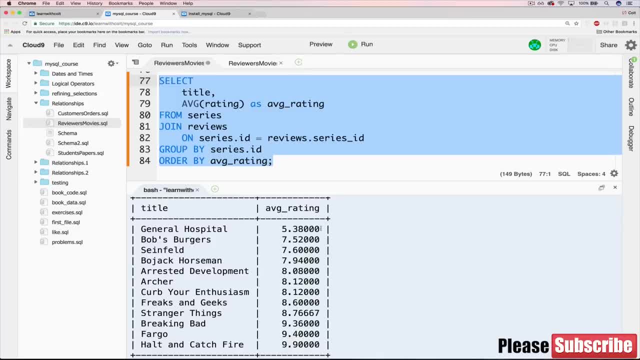 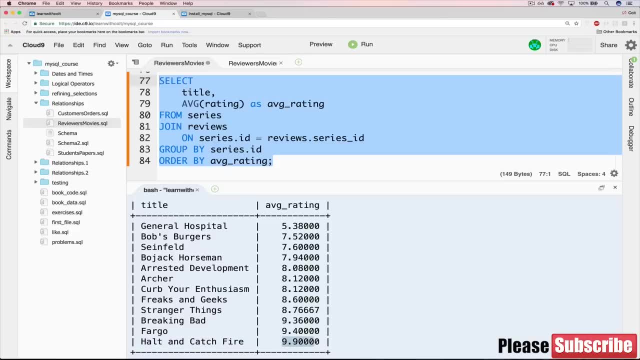 average rating. I'm sorry if that's a show close to your heart, But I want to highlight an amazing show that nobody watches, called Halt and Catch Fire. I mean, look at, this has a 9.9.. How did that even happen? I mean, who decided that? That's real data coming from real people? millions of 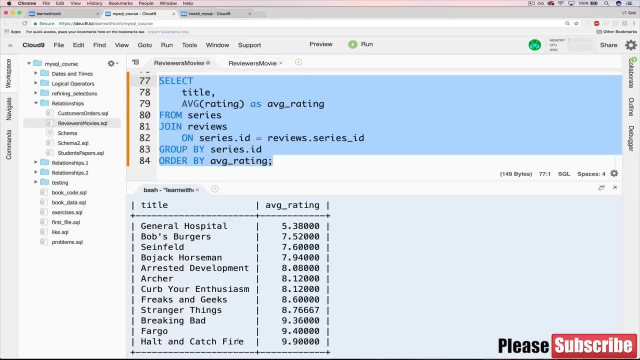 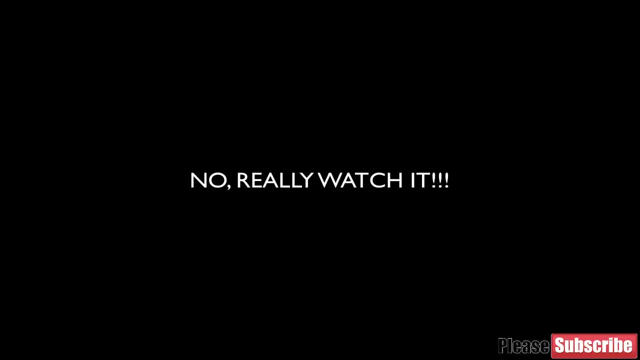 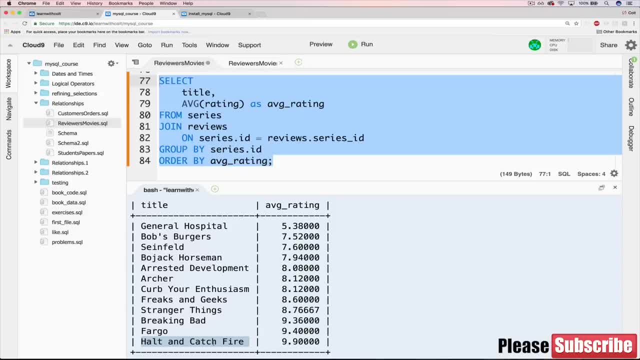 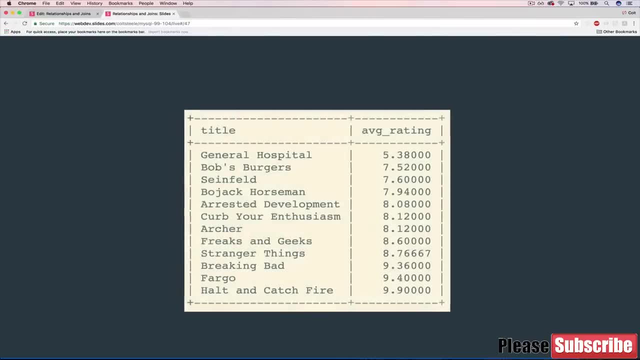 the internet, Although I will say season one is a little slow, but hang in there if you do want to watch it, All right. so we're moving on to our next problem in the next video, Watch Halt and Catch Fire, All right. moving on from the title and average rating challenge, we now have something. 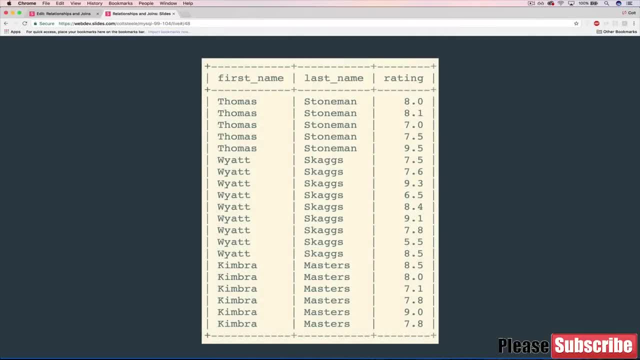 new. For the first time, we're working with reviewers, So what we have here is the first name of a reviewer, the last name and then their rating. So for every single rating that's been given, we want to have the rating. 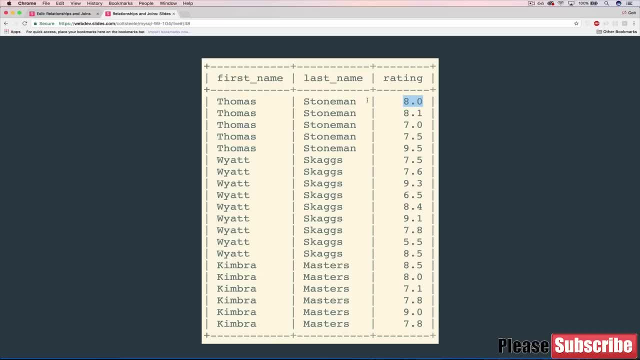 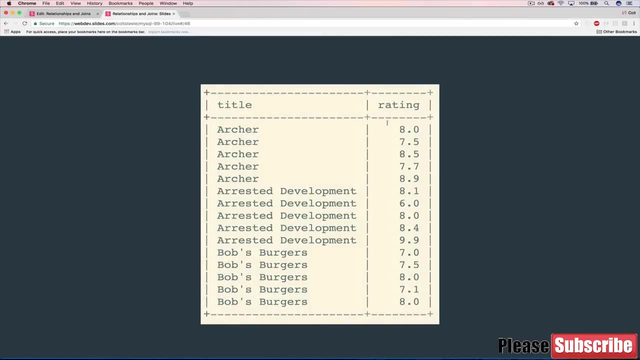 For every review that's been given, we want the rating and then the first and last name of the reviewer who gave that rating. So it's pretty similar to what we did up here with movies and ratings or series and ratings, except now we're working with the other table. So if we have these, 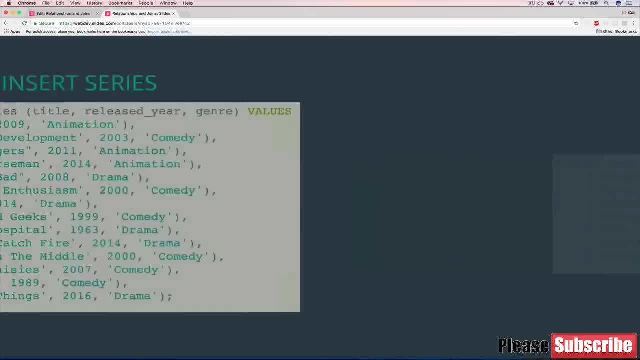 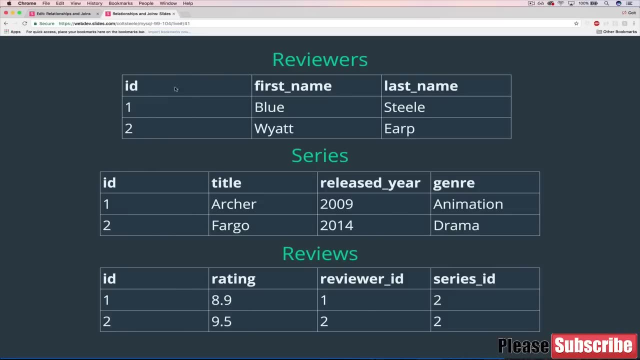 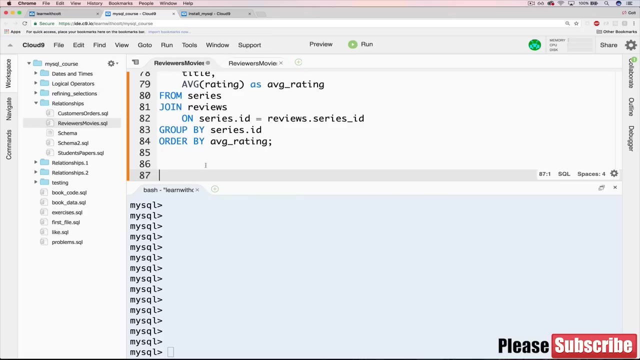 three tables. right, we've worked with- let's go back here. we've worked with series and reviews together. Now we're working with reviewers and reviews, So the average rating is going to be a little bit older too, So let's get started on this one. We will pop over here and just write. 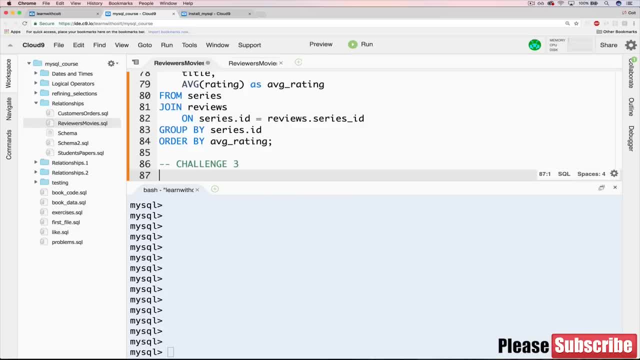 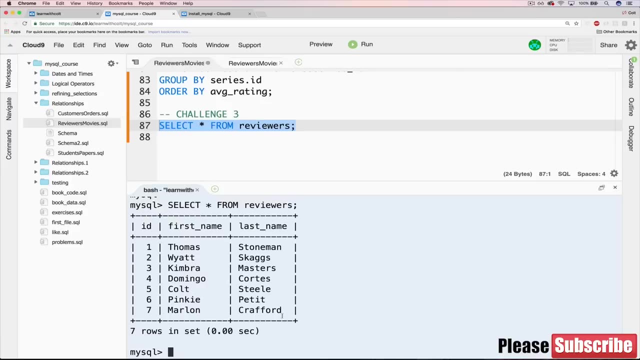 challenge three, obviously the most important part of this entire video. So we know we want to work with. let's start with reviewers. That's the first thing we want to work with. Let's take a look at those seven reviewers. Okay, so for every review that these reviewers have written, we want to see. 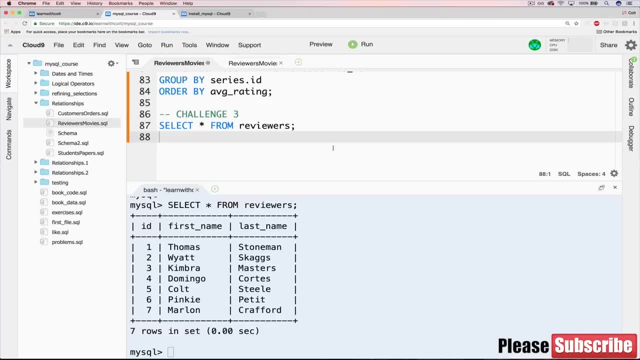 what they've written. And another side note: I deliberately put in a reviewer who hasn't written any reviews. We'll get to him or her in a little bit, but we don't care about that one in this case. So for this problem, we don't need to worry about that. Okay, so we've got select star from. 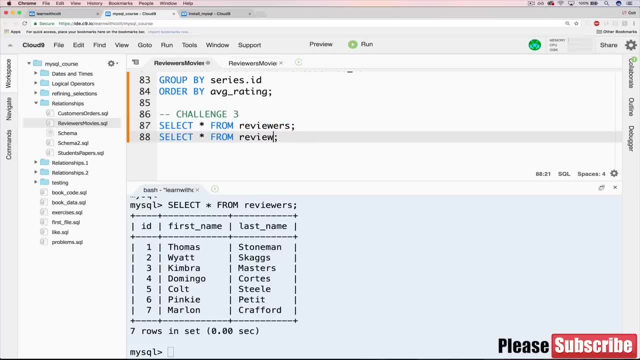 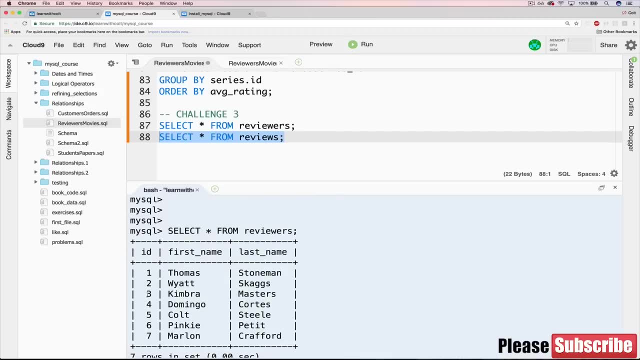 reviewers and then let's just do a select star from reviews And all we want to do is take these reviewer IDs- Let's take three for Kimbra and find all the matches where we want to put. the reviewer ID is three. So here's one, here's one, here's one. As you can see, Cloud9 is actually. 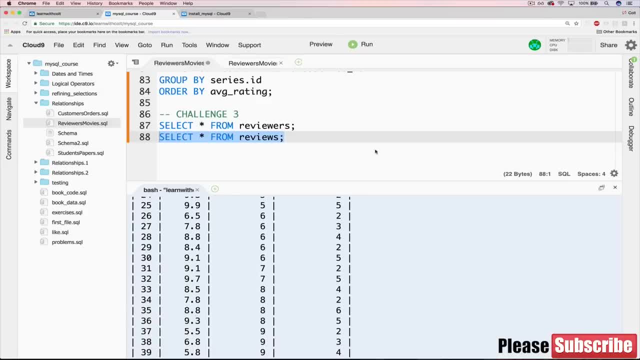 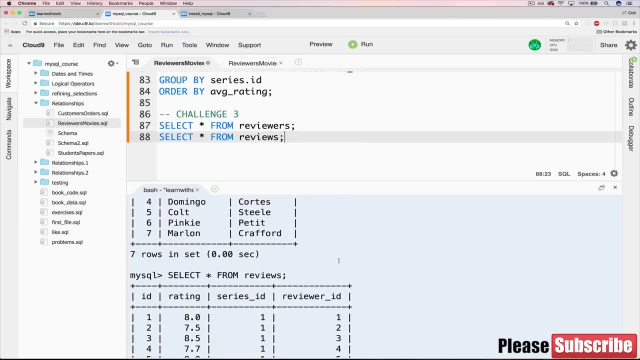 highlighting them for me, which is really nice. So we want to join on this right here. So we want to join between reviewers and reviews where reviewerid is equal to reviewsrootreviewerid. It's a lot of review. Saying that over and over is a bit of a tongue twister, So select. 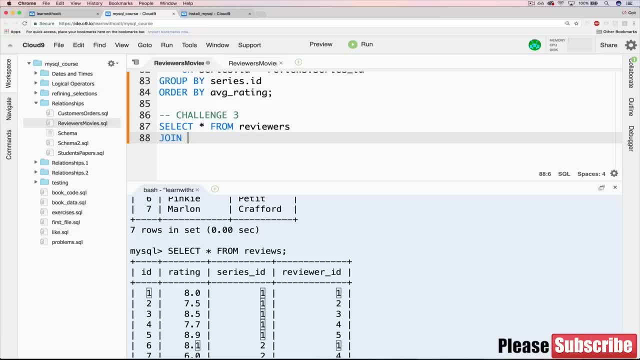 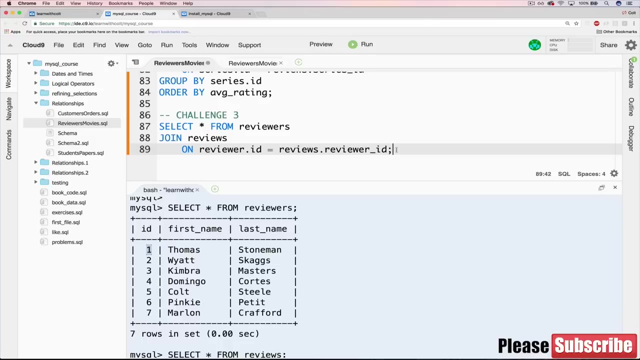 star from reviewers and we'll do a join reviews on and we want to do reviewerid equals reviewsreviewerid. It's a mouthful but hopefully it makes some sense. You're starting to identify the patterns behind these joins. We've been doing these a couple of times now, between the last. 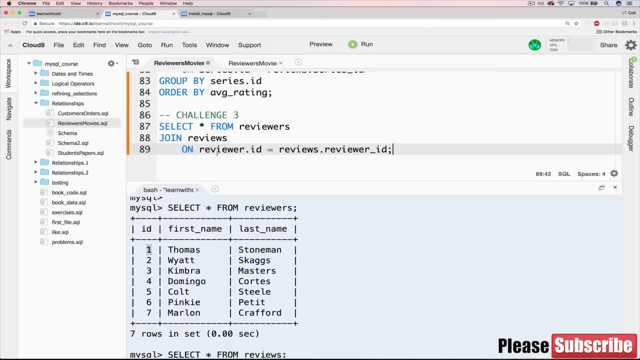 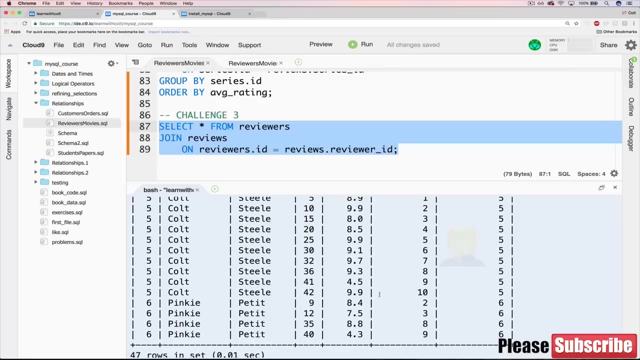 section and this section, So we're joining the two tables Where reviewerid is the same as, or reviewerid is the same as, reviewsreviewerid. And what do you know? I did the same thing without the S that I just warned you about. Okay, So now, once we fix, 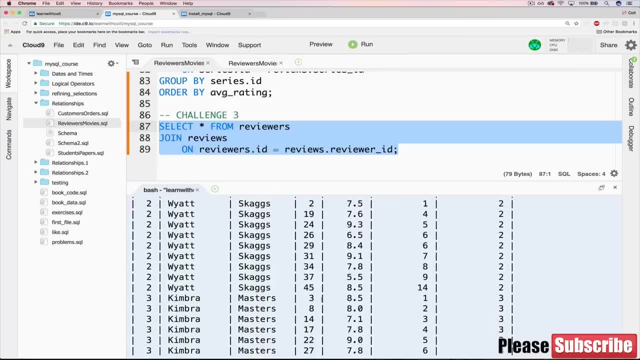 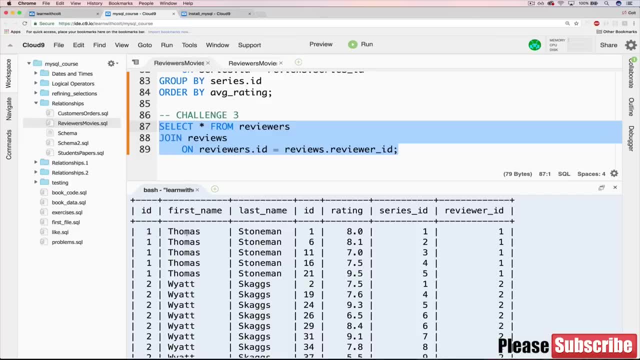 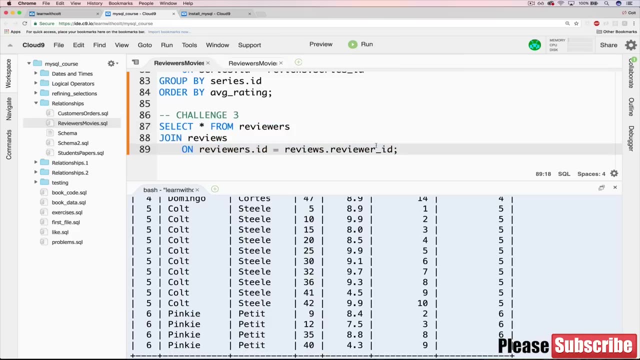 that we have a giant list. for every review that's been made over here, We have the corresponding first, last name and ID of the reviewer. So this is more information than we needed to get, because all we asked for was first name, last name and rating. So let's now whittle that down. So, rather than 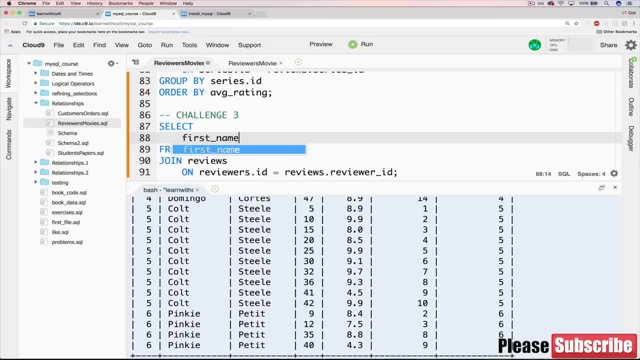 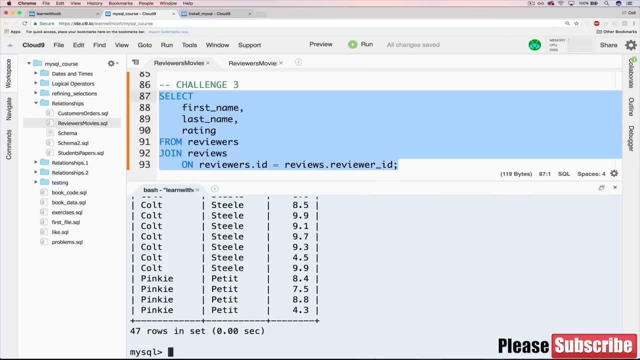 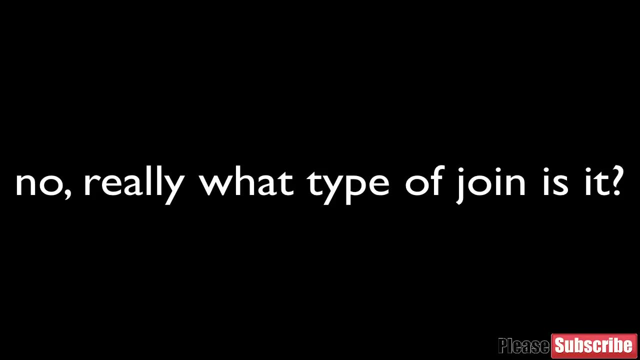 star. we'll select first name, last name and rating, Just like that, And now we get the right result. So I have a quick question, which is: what type of join is this? When we leave off the inner, it's still implied. So it's an inner join, the intersection of the both. 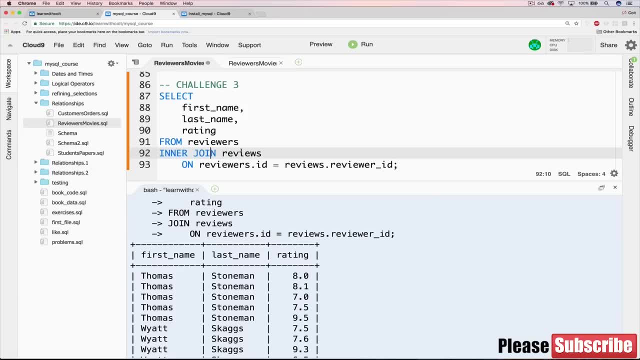 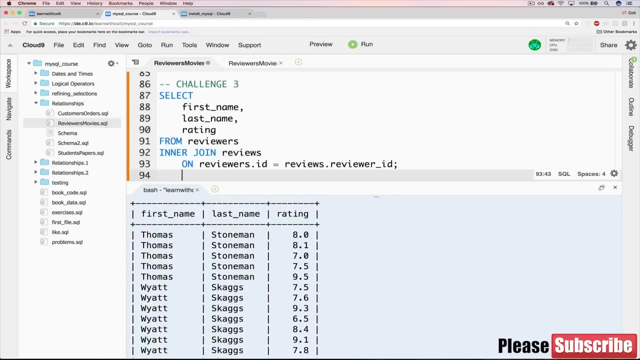 cake layers, those two circles, the two tables, and so, because it's an inner join, the order doesn't actually matter. so just to prove that to you first, here's what we had before, what you expect now let's do the same thing, but let's select from reviews. 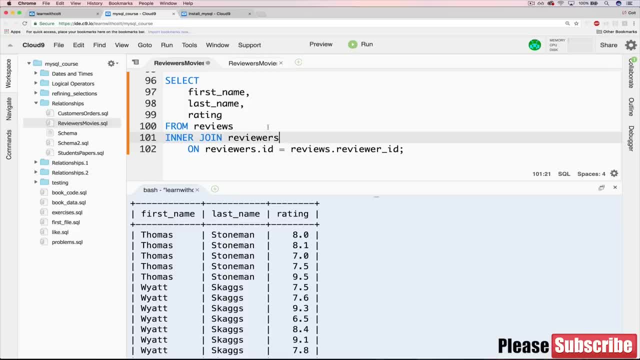 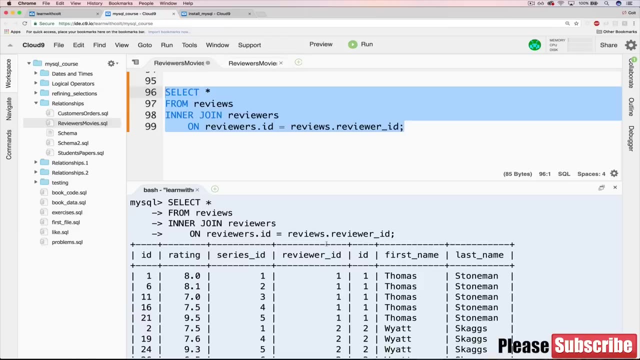 and inner join reviewers. okay, so if we leave this at star, which is what we had before, you can see that the order that our data is actually kind of printed in the basic sense when we use star is different. right, we have on the left the reviews and then the reviewers on the right, but when we're hands picking, 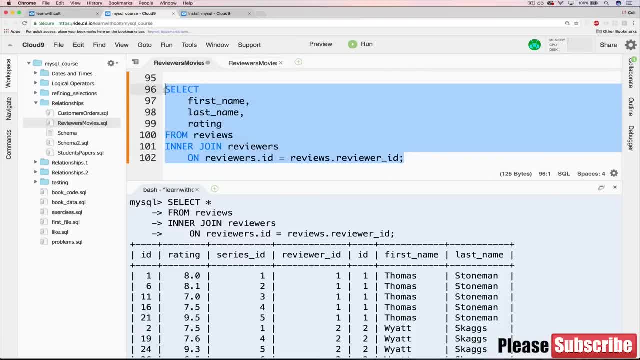 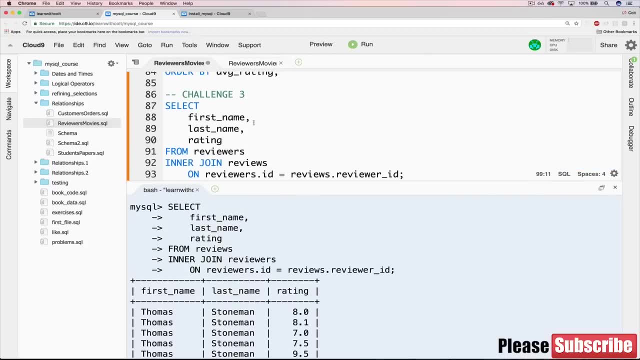 things that we want, like first name, last name and rating. it doesn't matter, because we're dictating the order. I'm saying I want first name, then last name, then rating. so as long as the data is in the right place- which both of these do- they're combined, they're in the right place. they're in the right place, they're. 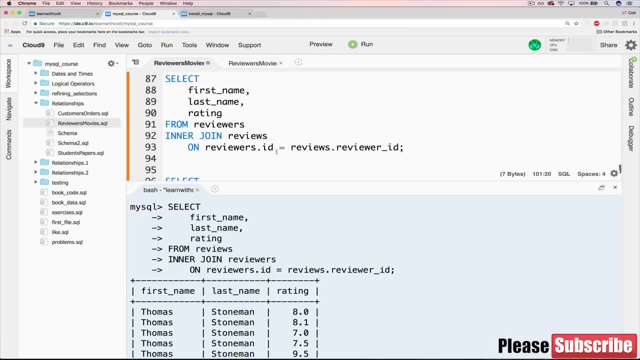 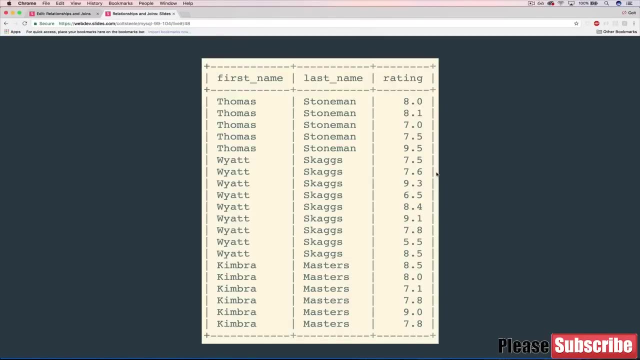 binding them. whether we're doing reviews- inner join reviewers or reviewers- inner join reviews, the same data is there, and then all we're doing is cherry-picking what we want. so both of these work just fine. okay, moving on to our next challenge, with the same data, something a little new and, frankly, 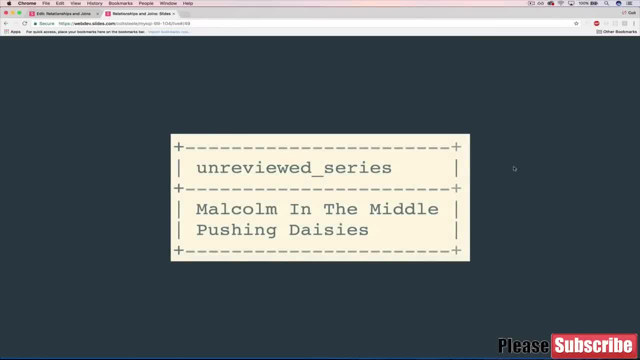 refreshing to see such a short table. so what we're doing here is identifying the unreviewed series in our database. so there are a couple that nobody has written reviews for, for whatever reason. I haven't seen either of these shows really. I've seen Malcolm, the middle maybe. 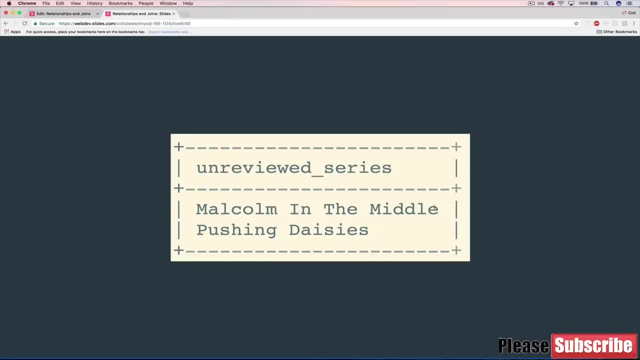 once or twice as a kid, but I don't feel like I can review it and apparently nobody else in our app felt that way. so we have two unreviewed shows and the point is not to cheat and to just, you know, use this information to find it. but 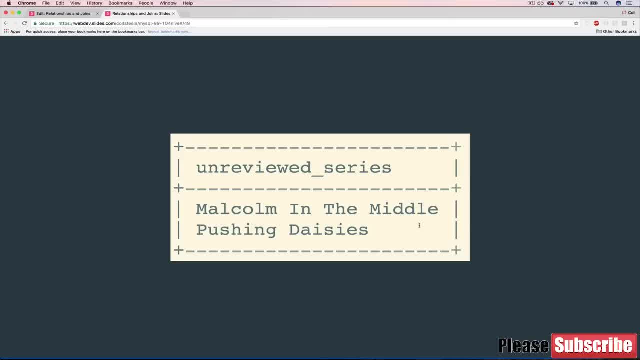 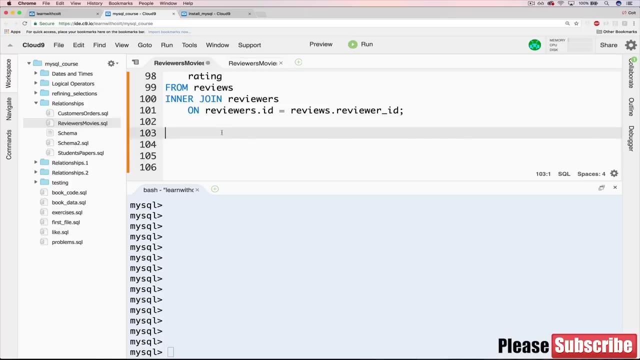 to actually find it based off of the data we have in our database dynamically. so how do we write? it's going to be a join. what type of join do we need to write where we can see what series have not been reviewed? ok, well, let's give it a shot. I'll hop over to cloud9 and we'll start with our 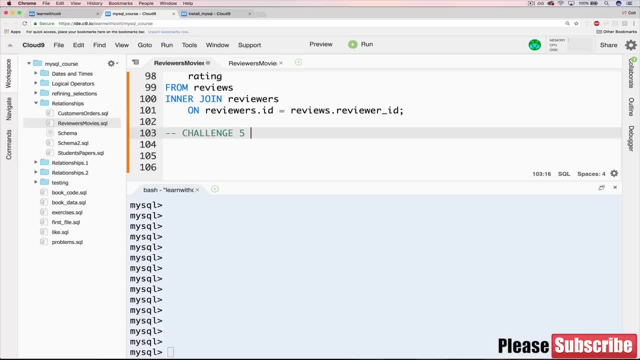 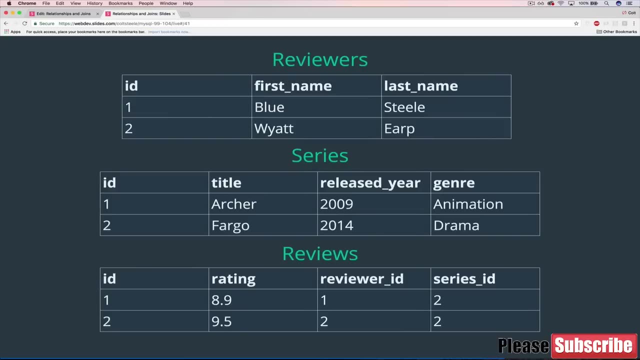 handy-dandy comment. we are on challenge 5 and this one is unreviewed series. ok, so what tables are we going to need to join here? so we've got, if we go all the way back here, we've got reviewers, get series and reviews and we don't need to care about. 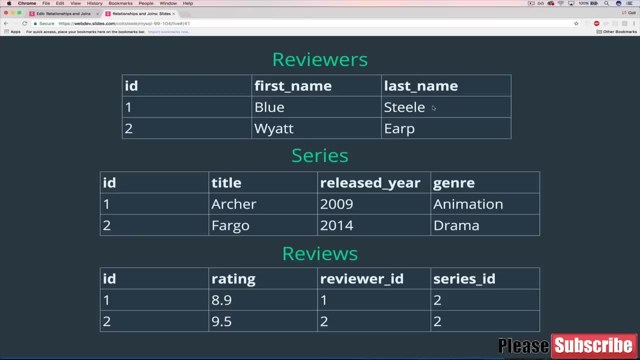 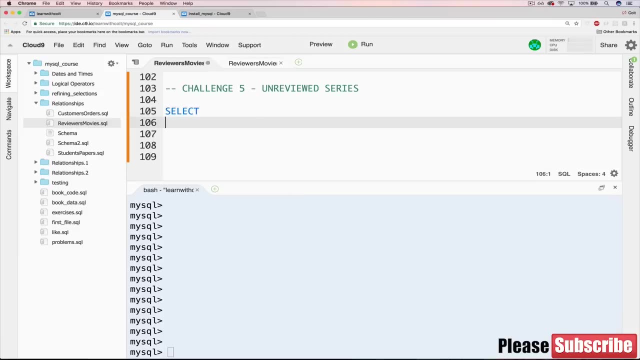 reviewers, shows. We don't care about names of who is reviewing things. What we care about is overlap or lack of overlap between series, TV shows and reviews. So let's start with a simple join Select and we'll do star from series And we can just start with that. Nice and 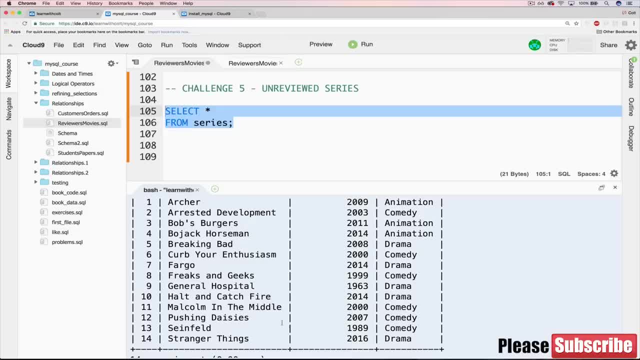 simple. It doesn't tell us anything. We have no idea which ones have been reviewed or not, So we need to join it with the reviews. So that's going to be join reviews on, and this is going to be our typical join. So seriesid equals reviewsseriesid, And let's make this. 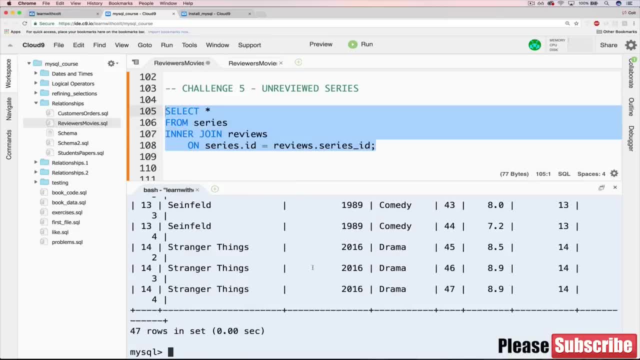 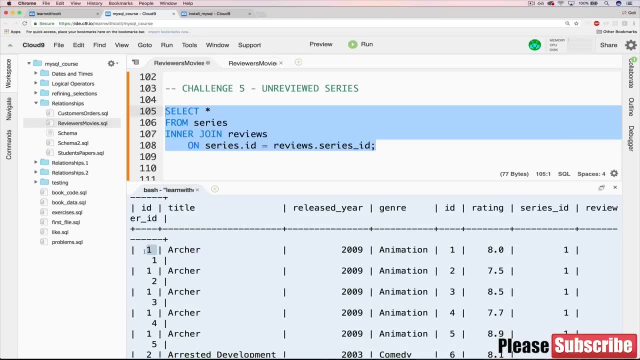 explicitly inner, just so we're clear there. And when we do this we get a lot. So let's kinda ammo over this. We see item review: right. We see Archer with an id of one. It's been reviewed with 8.0, 7.5,, 8.5,, 7.7.. But there's a problem here which is it's not doing. 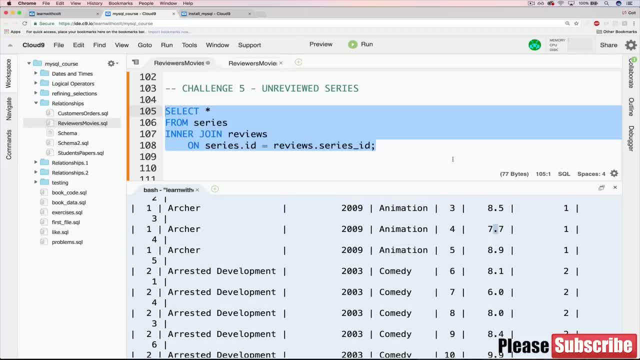 what we want. We're not even really composed to what we want. In fact, we're ignoring the data we want because this is an inner join. So this is only finding the exact intersection between reviews and series. So wherever they overlap is what it's saying is good from here. 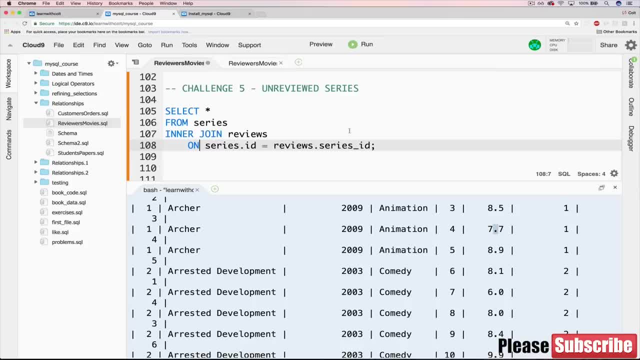 is what we're seeing. But we also want to identify where they don't overlap, because that tells us that there's not a review for a series. So what we want to use is a left join. So hopefully that makes sense. Why? Because on the left if we have our series right. 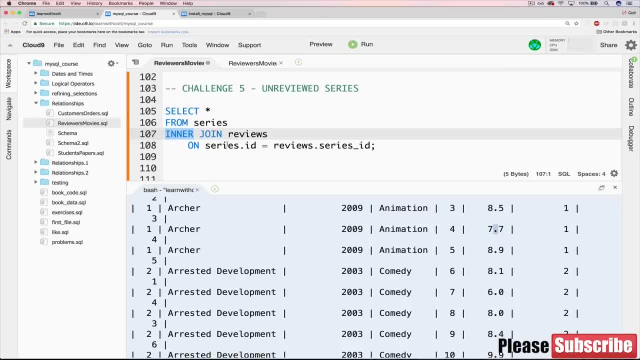 we have all the series, some of which have matches, some of which don't, and we do a left join. it's going to take everything from the left, including the ones that have no reviews, and it's still going to stick them in the join table, but it's just going to fill their values. 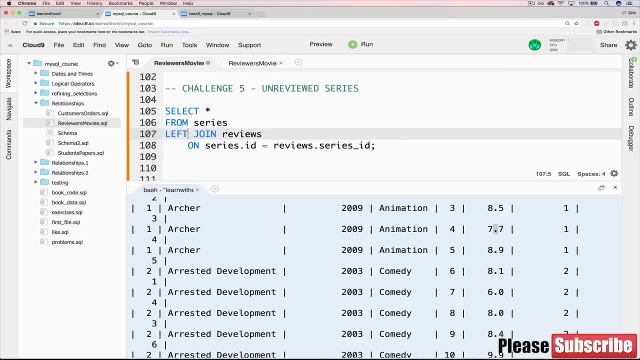 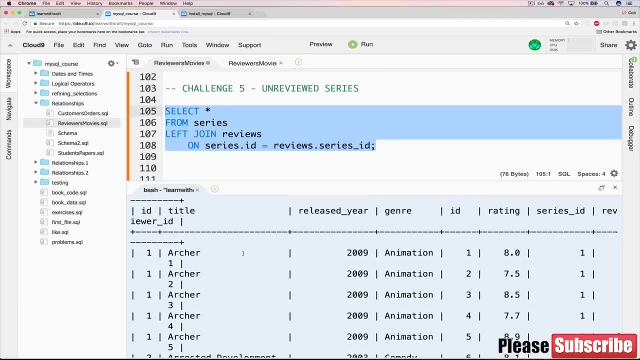 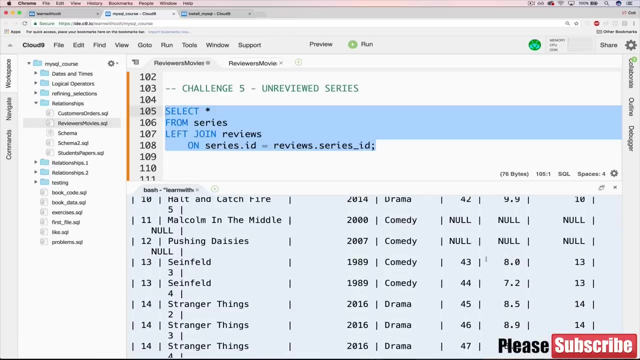 with null, So we'll be able to identify that. So if we change it to left join and we scroll through some of this, you'll see somewhere. so we've got Archer with all these reviews over here. If we keep going down here we go. Malcolm in the middle has null. 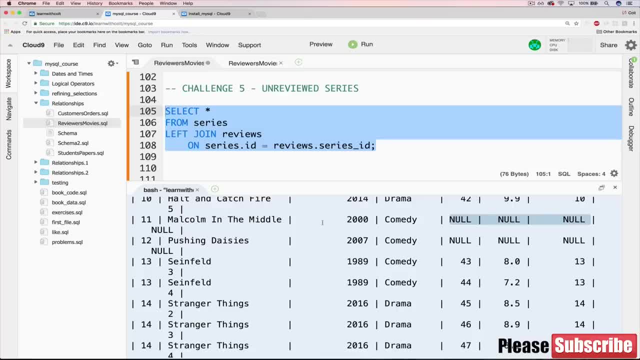 because there are no reviews to match it with, But because we did a left join, we still get Malcolm in the middle and Pushing Datas, which is also- or Pushing Datas, geez. Pushing Daisies, which is null, null, null, null as well. 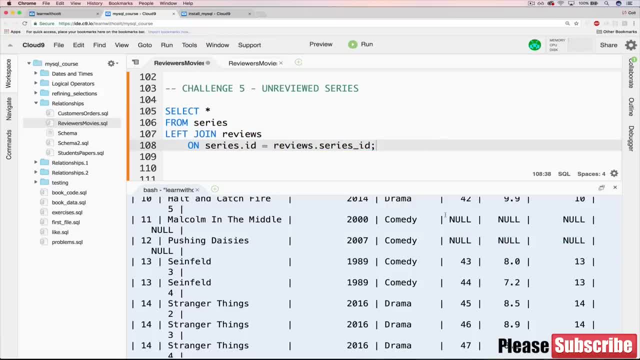 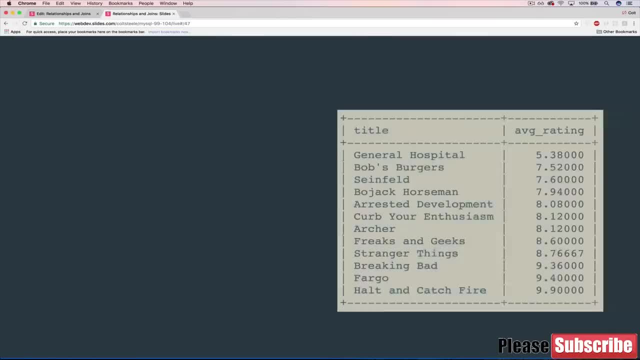 So we can use that to our advantage, because wherever we see, null means that there are no reviews. So what we want to do first, let's whittle it down a little bit. What we're looking for at the end is just title, but let's start by just doing. 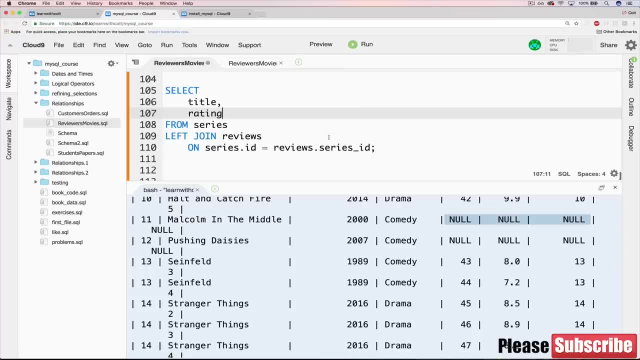 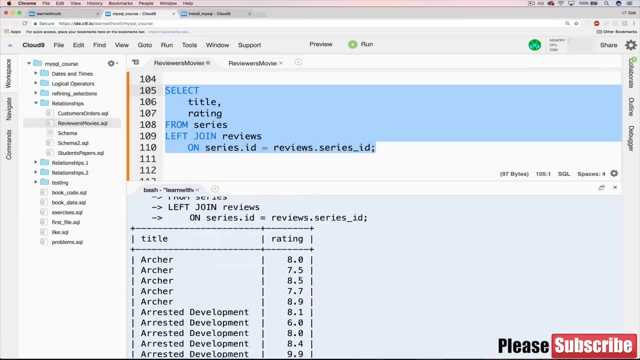 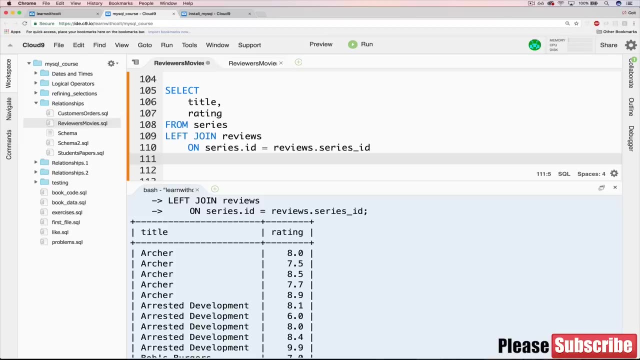 title and rating. Let's do that So it's a little easier to see. Okay, So now what we want to do is only work with the data where there is no rating. So that's actually quite simple. All we need to do is use a where and then we can pick rating. for example, equals and. 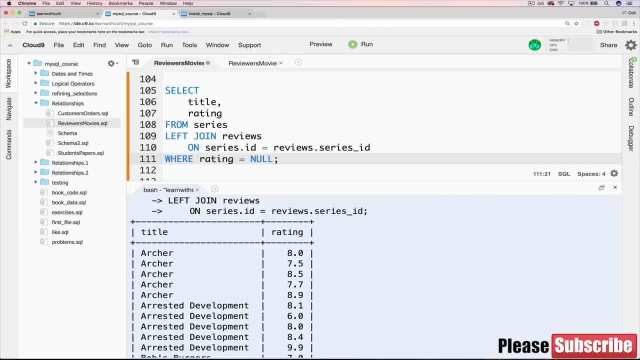 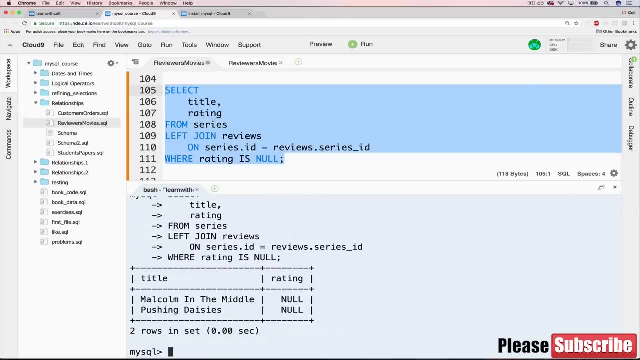 we can't say equals null, because that's problematic, Remember. what we need to do is do is null, just like that. So let's try this now and you'll see we only end up with these two title and rating. 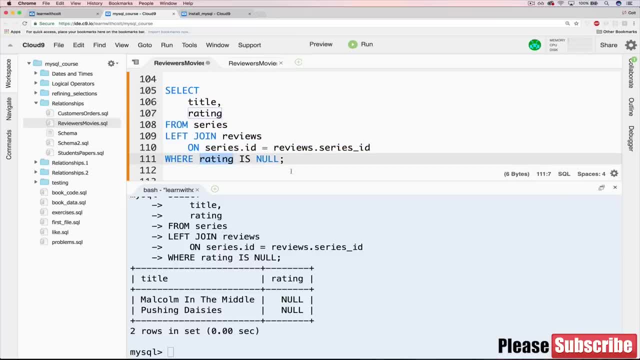 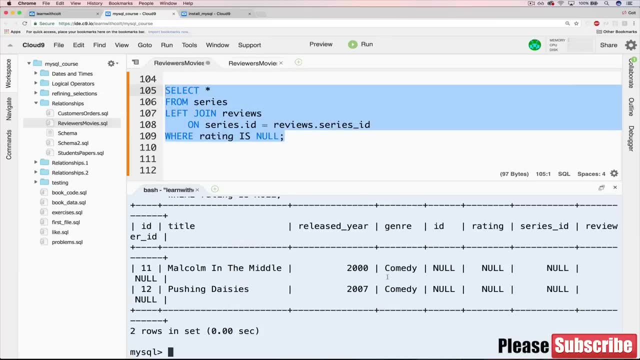 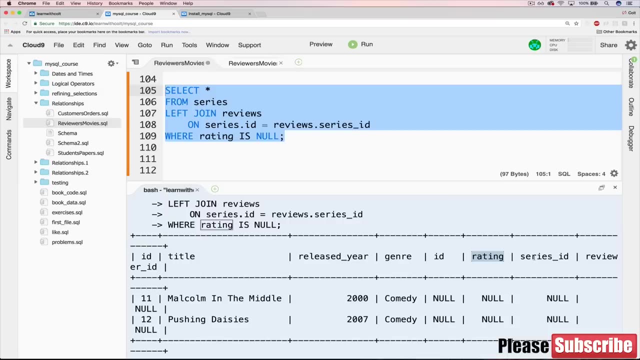 And we don't have to do rating, by the way, because there are other fields that are null. If we go back to star, there are quite a few things that are null. We could have done ID, although this is reviewsid. we could have done rating series ID or review ID or reviewid. 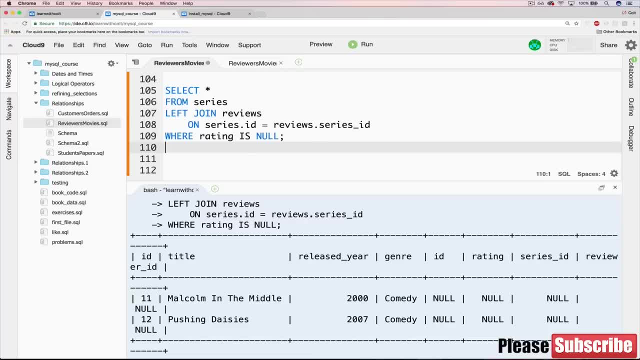 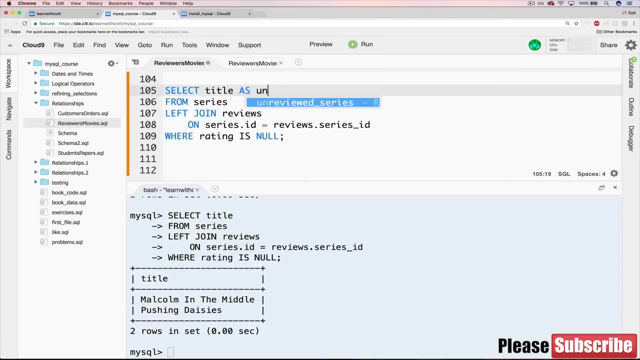 Okay, Okay, But it doesn't matter which one we pick in this case. So let's go back and all we actually want to do is select the title. That's all we need here. Paste that in. Okay, Only thing that's missing is the alias. so we'll do. select title as unreviewed series. Copy that in. 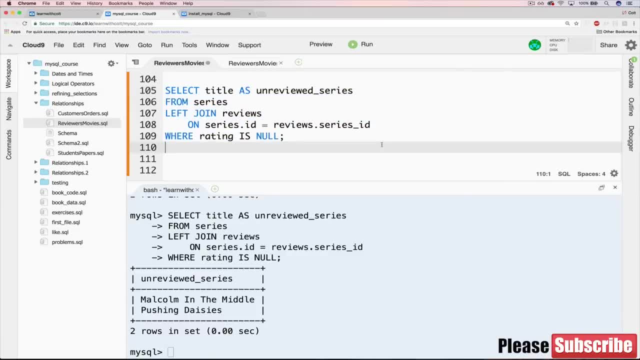 and it works Okay. So the key thing here was that we used a left join. We wanted to highlight those discrepancies. This is a use case for a left join, Where you want to see where there is an overlap. So hopefully that helps illustrate a bit more. 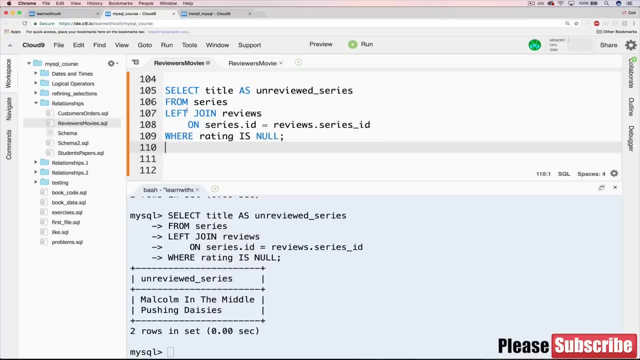 the difference between inner and left joins, Because if we had only done an inner join here, we wouldn't get the result we want, We wouldn't have any nulls, So this wouldn't select anything at all. Okay, So next up we have another nice clean table. just three results And, as you can, 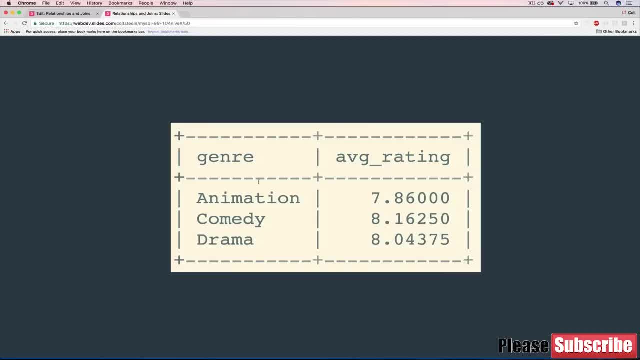 see, what we're doing here is grabbing things based off of genre. So we only have three, fortunately: Animation, comedy and drama, And then what we're doing is computing the average review, or the average rating for each of those genres. So this will be a little similar to what we've already done earlier. 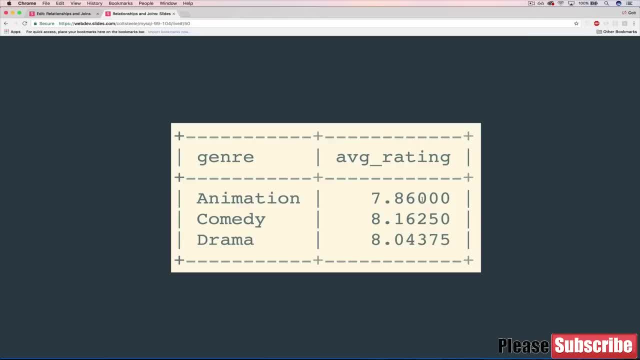 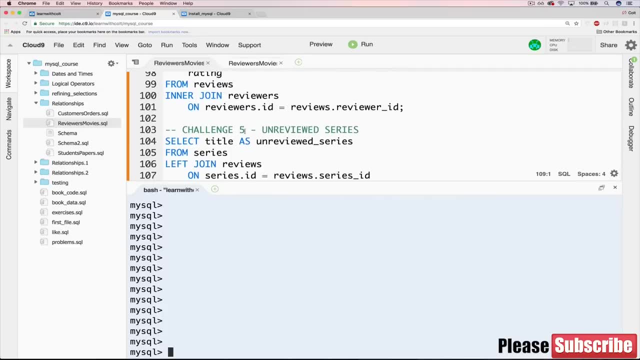 in this problem set. The main difference is that we're working with genre now rather than just the title of a given series. Okay, One thing: I need to correct the record here. I called this challenge five. I was wrong. After four. after three comes four. Now we're on. 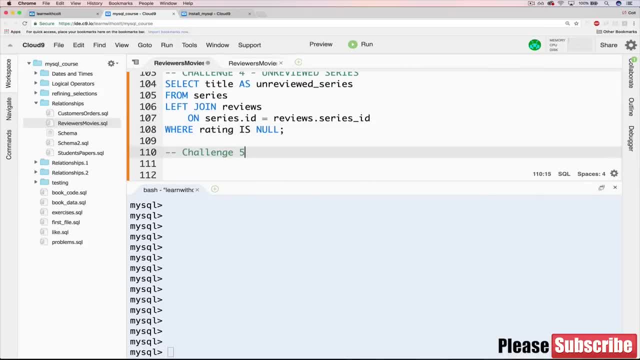 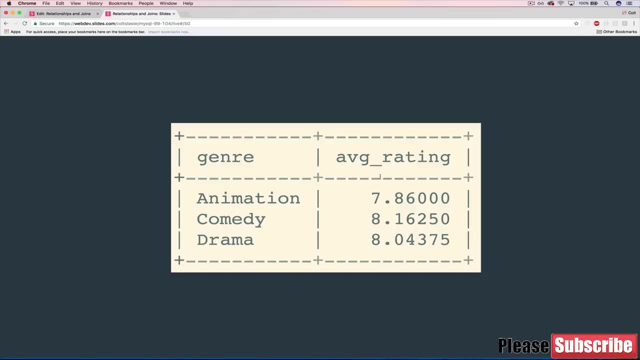 challenge five, Okay, And we'll just call this genre average ratings, Okay. So, to get this information from our three tables, the two that we need to identify that we're working with are the series table, because that's where our genre information is stored, and then the reviews table, That's. 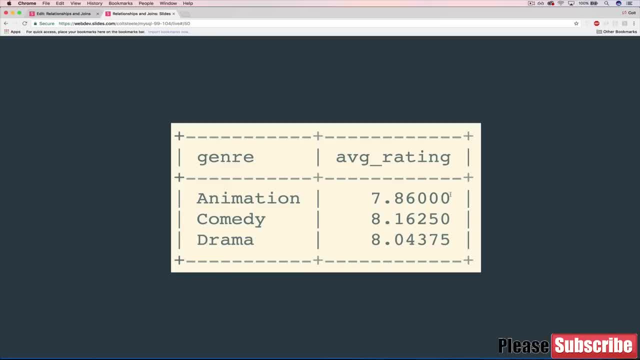 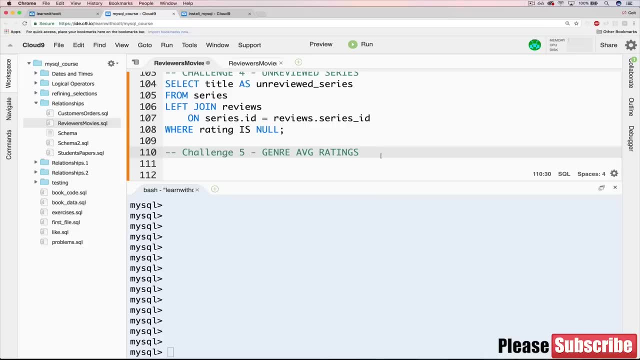 where our ratings information is stored. So we don't care about the reviewers, the people who reviewed them, That doesn't matter. All we need is the genres and then the ratings, So we can start with either one. Let's start with star from series, just like that, Okay. 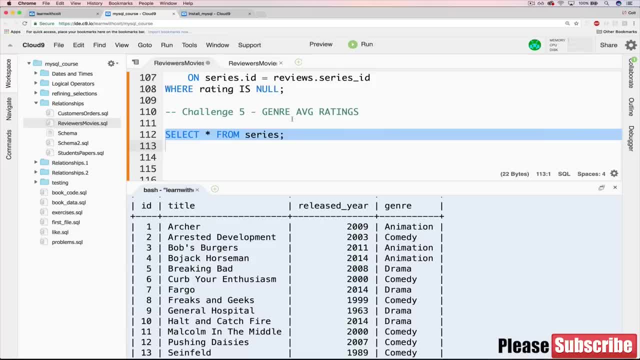 So all we're going to want to work with is the genre portion, but we're going to need to join with the reviews table, So we'll just do that now: Select star from series, join reviews. Hopefully this seems familiar now On seriesid equals. Okay, So we're going. 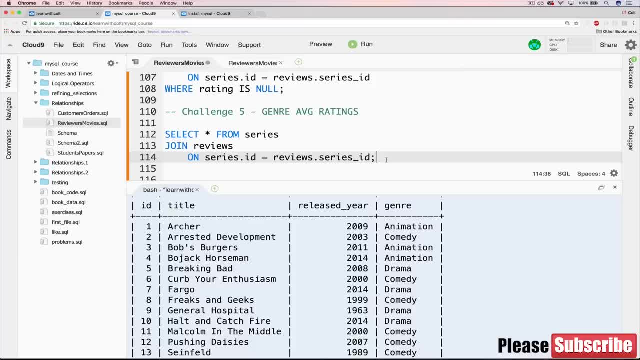 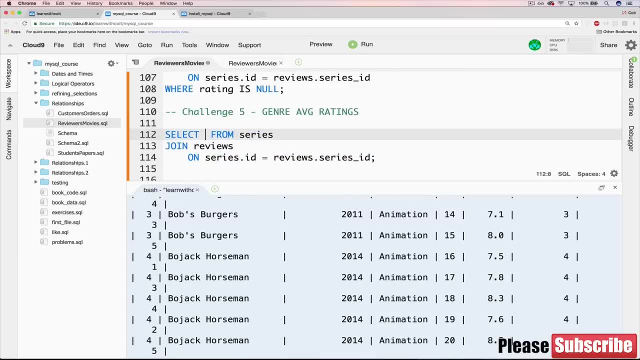 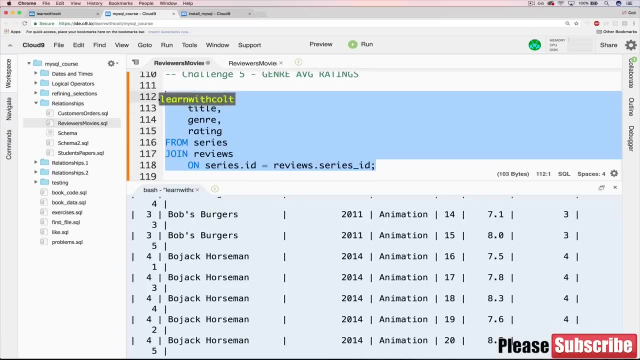 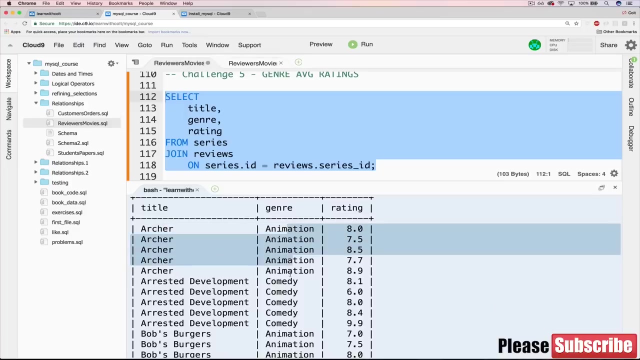 to get reviewsseriesid, And if we leave the star in there, we're going to get a lot of stuff. So we don't need all of that. Let's just pick out a few things like title, genre and rating. Okay, So now we can see. we've got, you know, all the ratings for Archer. 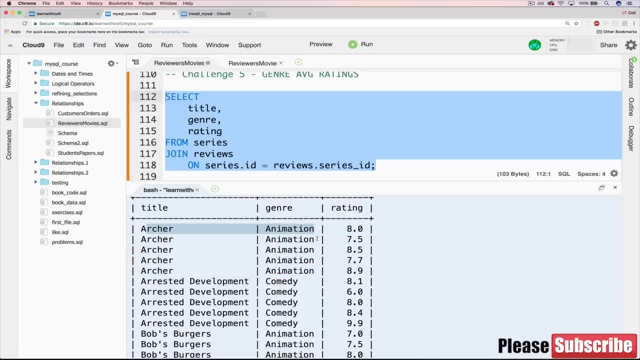 all animation, of course, because they're the same exact row here with a relevant rating Appended. So we've joined them together. It's an inner join, And that's what we want. We don't want to be working with- uh you know, non-existent ratings. We don't want. 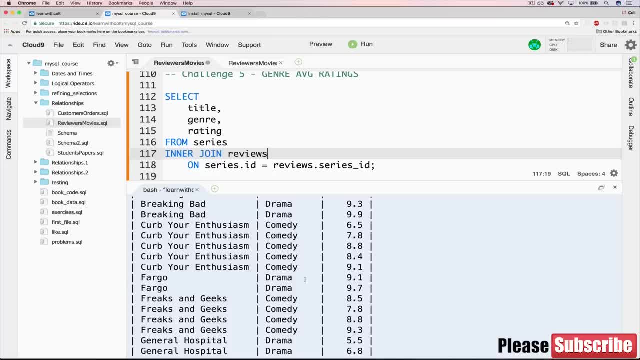 to take. let's say what was it? Uh, pushing daisies which didn't have any reviews. Well, that's a comedy, I believe. Maybe it's a drama, I don't remember. but whatever it is, we don't. 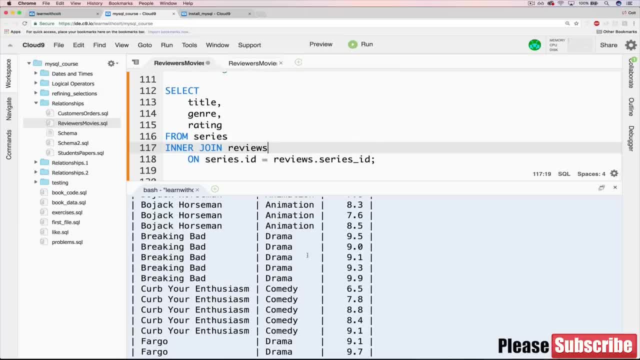 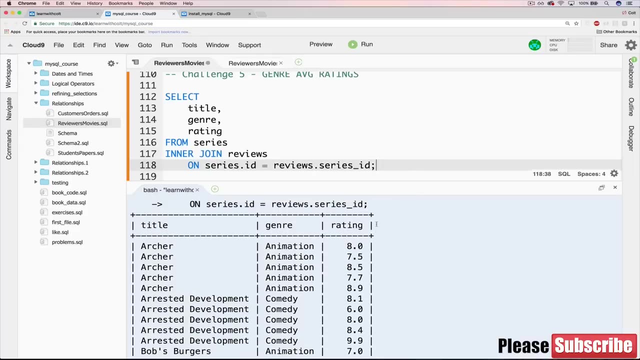 want to try and average null into the average rating for drama. So the average rating for comedy. We don't want to do a left join. You want inner? Okay, So we've got this on series ID: blah, blah, blah, blah blah. Now all we need to do is group things by genre. That's what. 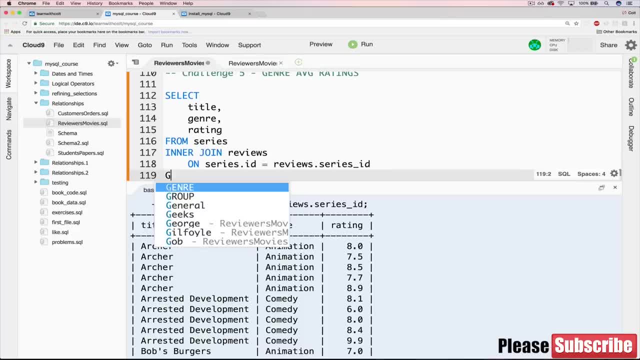 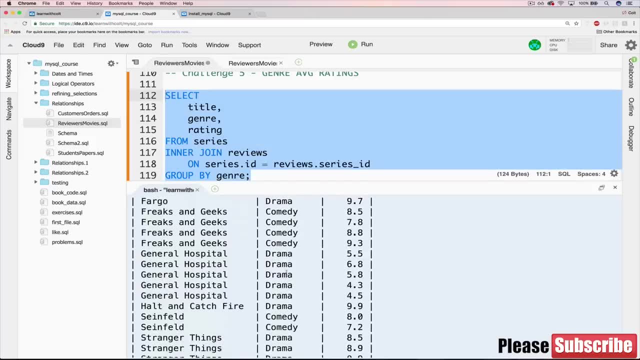 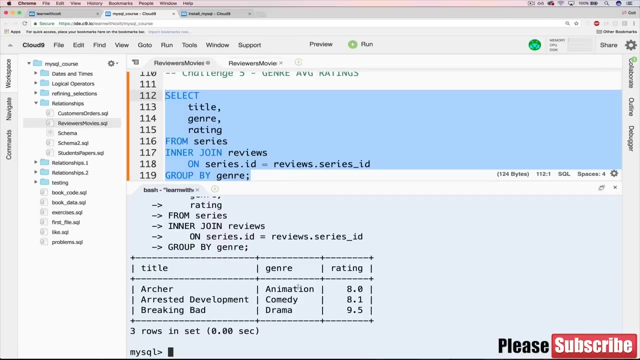 we're trying to do here, rather than by title group, by genre, And if we do that, we should see. this is immediately reduced down to three rows, Although remember that it's just kind of hiding all the data that lies beneath. So we have animation here, Um, but it doesn't mean that there's only one, It's just that. 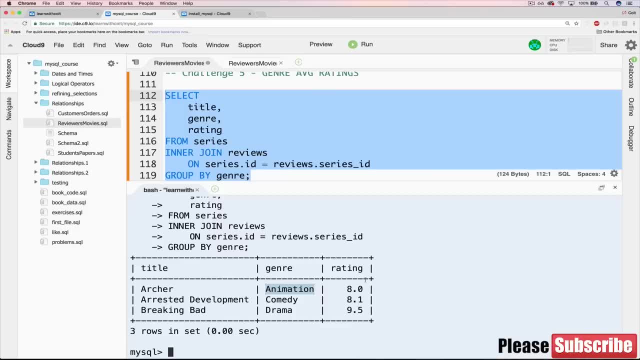 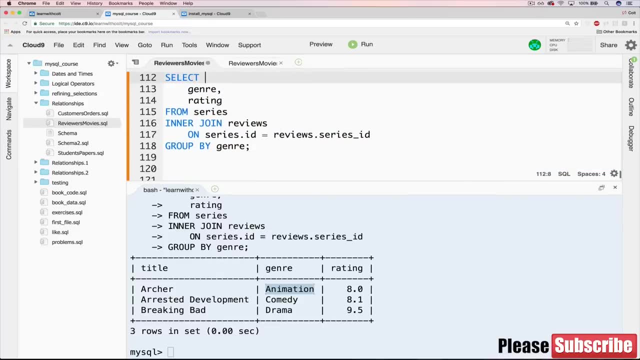 group by when you, when you use a group by, it's displayed in a very weird, awkward way. that I think is kind of confusing. but what we want to do is, rather than we can get rid of the title to, um, rather than just genre and rating, we just want average rating and 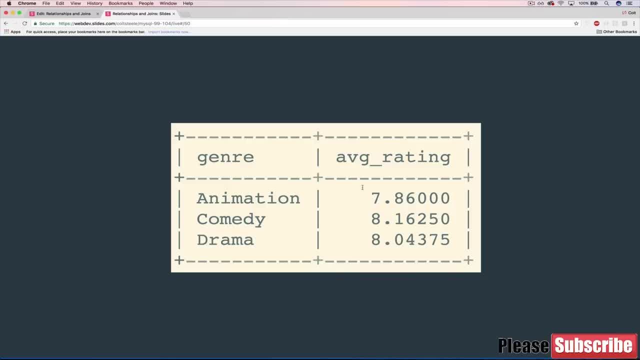 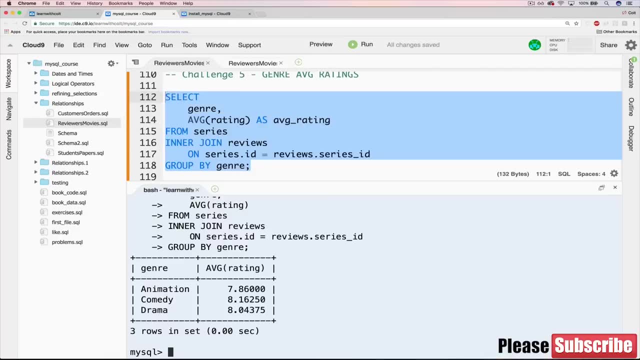 that should do it for us. We get the average ratings and there's an alias. So Yeah, Yeah, You can add that in like that and that's it. So now we get animation. It's the lowest rated, still quite high. Comedy is the highest rated- 8.1- and drama is right in the middle. 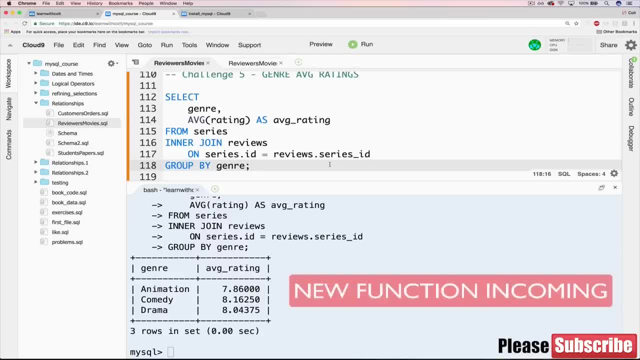 8.0.. And I suppose this is as good a time as any to introduce the round function. We haven't used it yet, but we're getting a lot of decimals here and we don't. we don't care about them. Let's just round it to. let's do two decimal places. 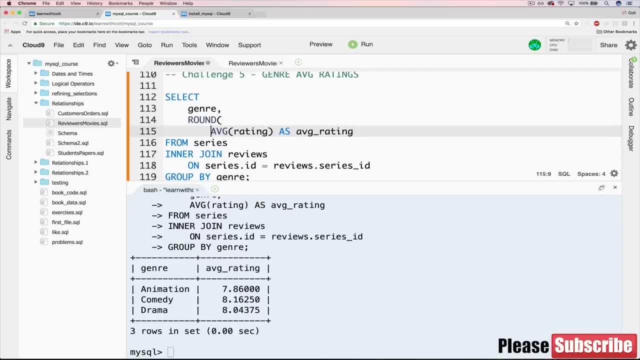 So it looks like this round, and I'll do it on separate lines here. So we have round average rating, but we don't just say round average rating. We have to supply what we want to round it to two digits for us, And then we'll use ads average rating. So I could. 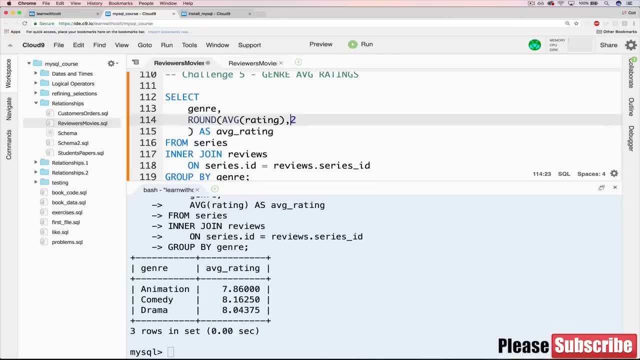 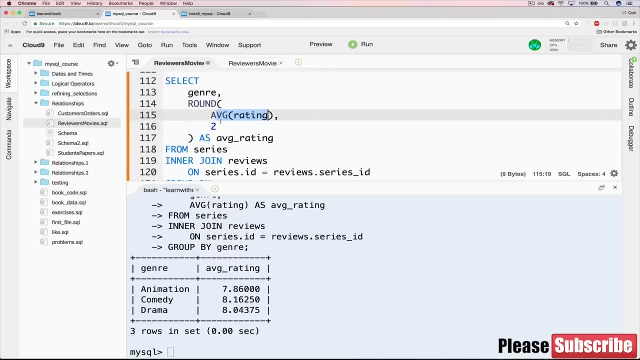 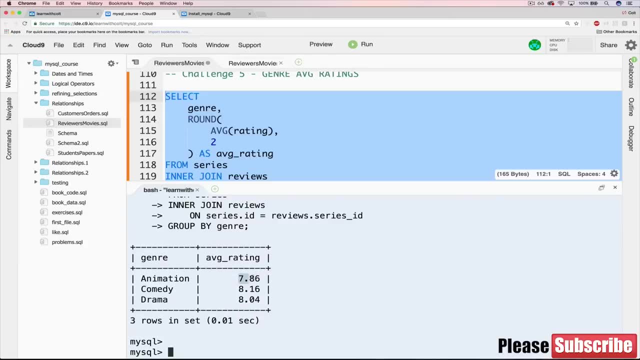 It's a price we pay, Okay. So round the average two digits and call it average rating. Now let's double check that works, And there we go. much easier. You didn't have to do that, of course, but your figure, there's a good thing to show, Okay. So next up we have a. 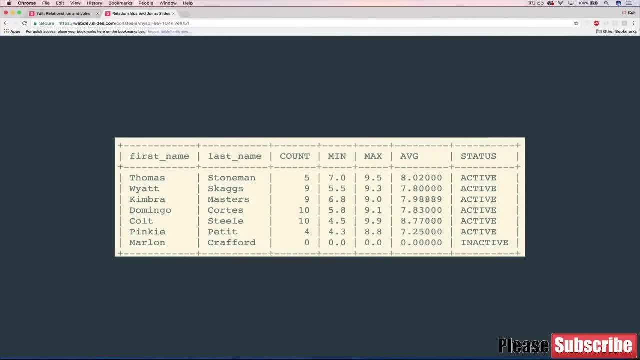 return to these long, annoying tables with quite a few fields. on this one, This is sort of like analytics for our reviewers, And what we're doing here is compiling statistics on them. So, Thomas Stoneman, How many reviews has he written? Five, Okay. What's the minimum he's assigned? 7.0.. The 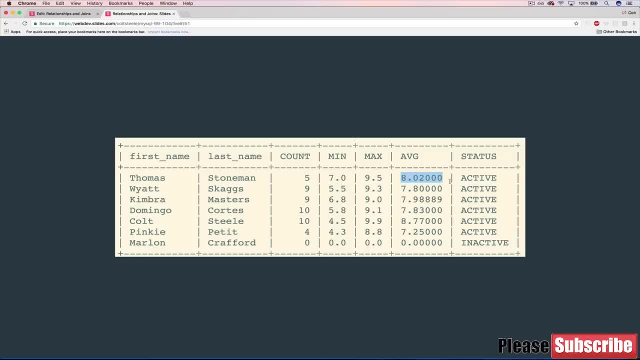 maximum review is a 9.5.. His average is 8.02.. And then a status, which is saying that he's active And that's determined based off if they have, if the user has any reviews. So Marlin craft Crawford has zero, So he is inactive, but everyone else is active. So we've got. 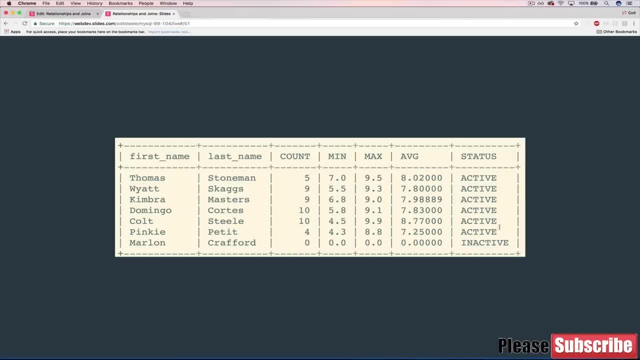 a lot of pieces here and probably the most crucial thing to point out Is that we have Marlin Crock Crawford, who has zero reviews, which we need to pay attention to. We have to pay special attention to that because there's not going to be a natural. 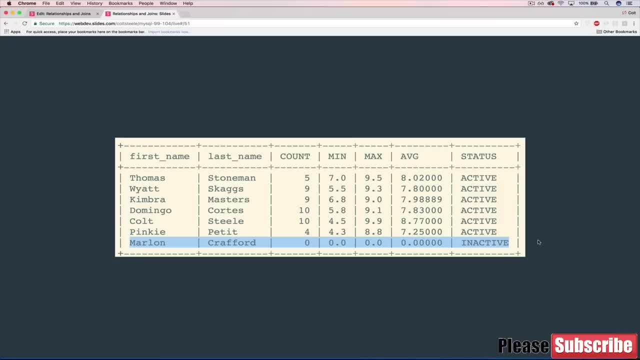 join. if we do an inner join, So we'll need to do a left join, which will highlight the fact that he has no reviews, and then the rest is not too difficult. Count min, max average should be pretty comfortable with that status. Hmm, We need to do some logic there. So let's. 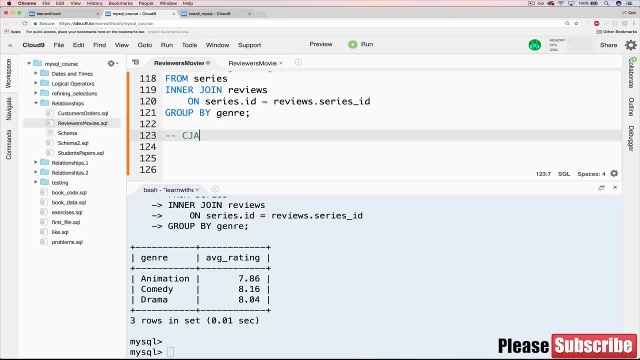 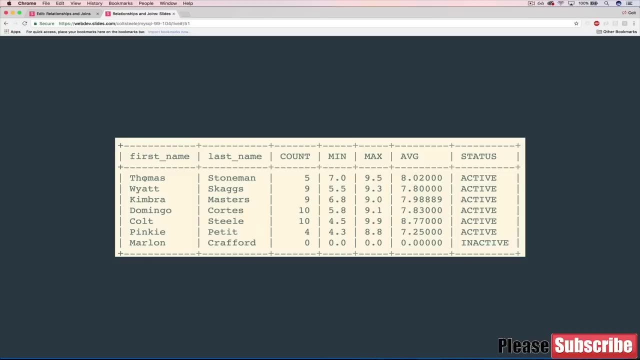 start, Okay, By adding in challenge six. we'll just call this reviewer stats, Okay. So the tables we're working with: we've got the reviewer table, which is where we're pulling things like the name, And then we've got the reviews table, which is where we're pulling count min. Well. 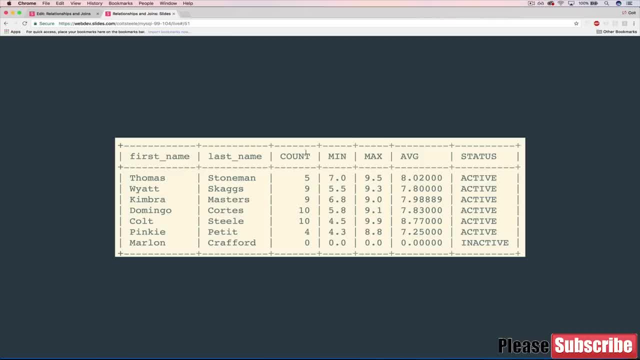 that's where we're pulling the, the actual ratings themselves, And then we're basically getting this data from there. So we don't need to worry about the series Table. we're not working with that. We will be in the next. uh, the final challenge here. 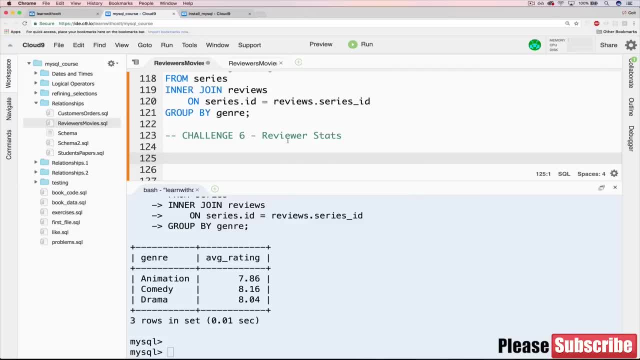 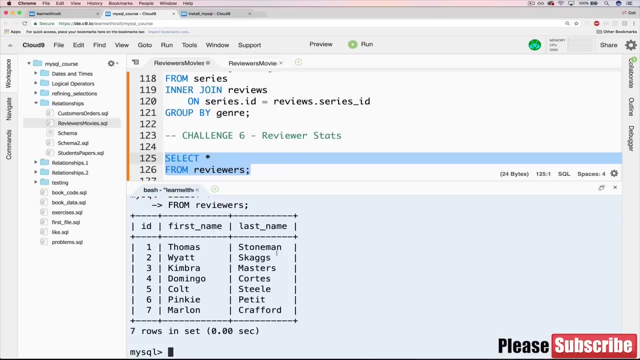 We're going to put all three together, but in this case we're not, So we'll start with a select star, or let's just do. well, we'll do star to start. Select star from reviewers. We get all of our reviewers here. Perfect, We want all of them. So that will be the left. 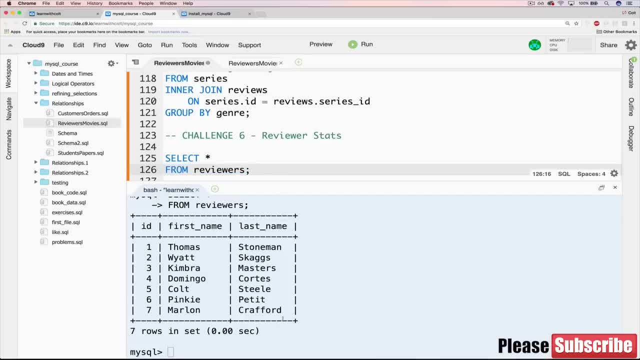 part of our joint. If we remember the two circles a and b, this will be circle a right here. We want all of this to show up, even though Marlin doesn't have any reviews, Then we're going to do a join. 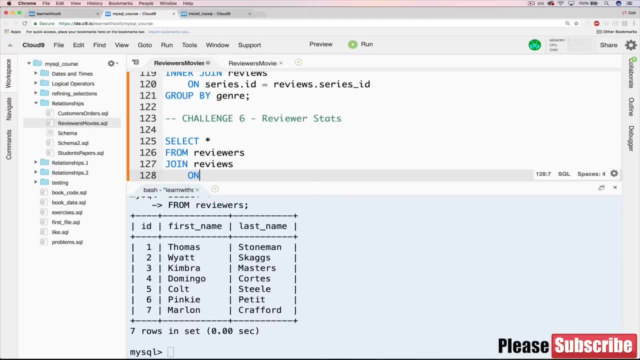 Join reviews on reviewersid. so where the reviewer ID like this- 1,, 2,, 3,, 4,, 5,, 6, is equal to the reviewsreviewerID, And then in the case of Marlin, 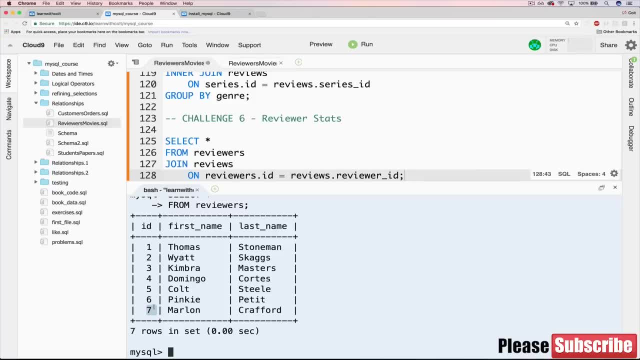 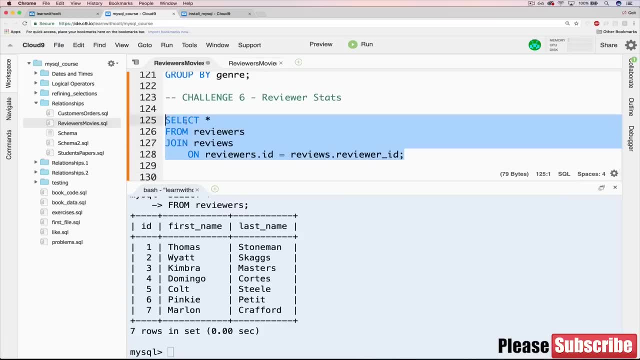 there is no reviewerID equal to 7 in the reviews table, so we'll get null, null, null and so on. Okay, let's try it. And if we take a look at the results here, we don't get those nulls. 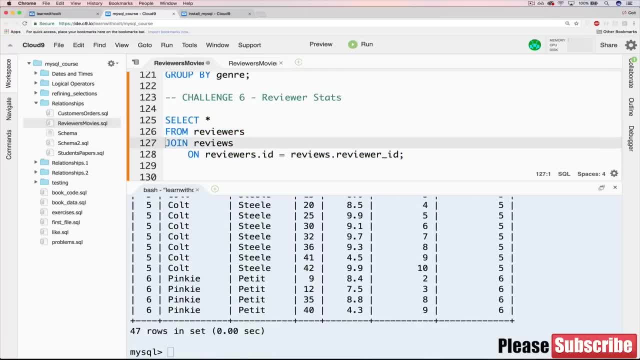 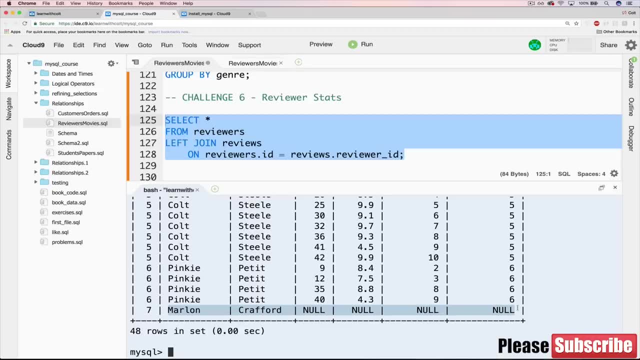 and that's because we didn't specify that it's a left join. We left that off And now at the end we have Marlin Crawford- null, null, null, null- which we'll need to make use of to do things like this. 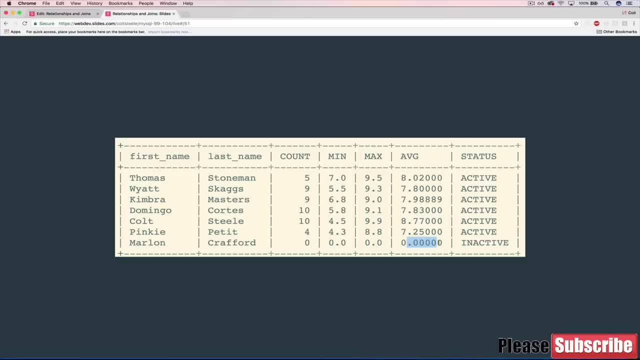 where we have 0,, min, max average are all 0, and then inactive. So we'll have to kind of make special exceptions for Marlin or for anybody with null. Okay, so now let's start whittling down what we need. 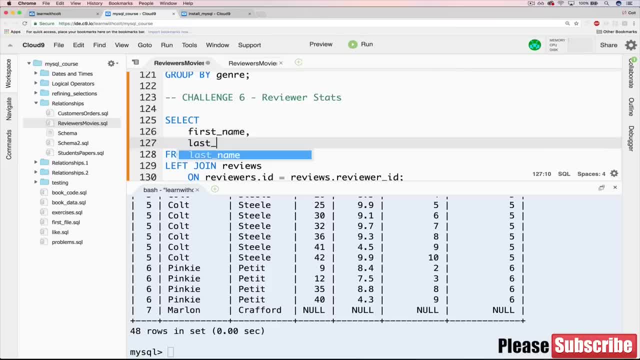 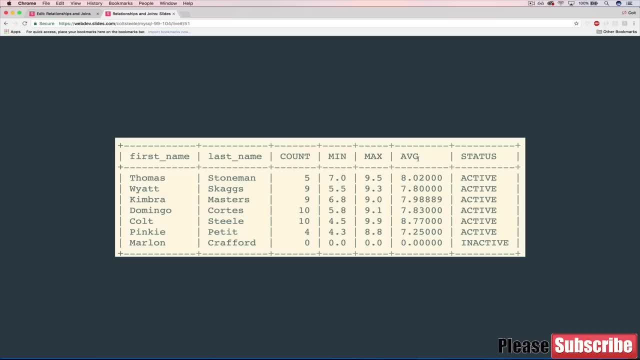 We want first name, We want last name, So what we have here right? Then we want things like count, min, max and average, which require us to group by. But let's start by just putting rating here, without grouping. 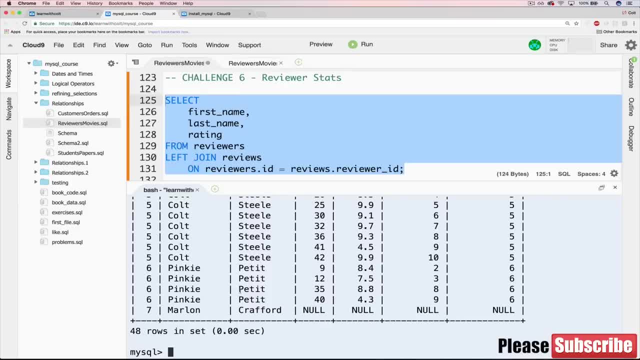 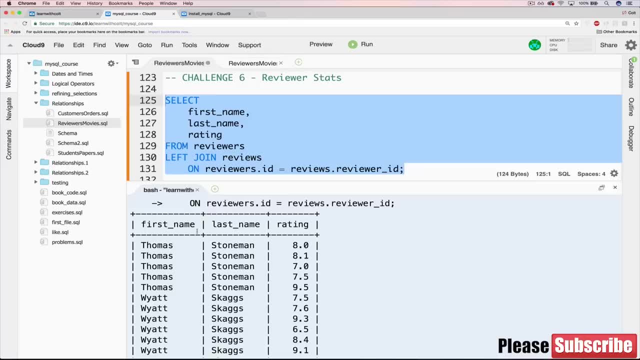 And just verify what we need exactly. Okay, so here's all the reviews And we want to group them together And we could group based off of first name and last name, but that's not guaranteed to be unique, of course, so it's better to group based off of the reviewer's ID. 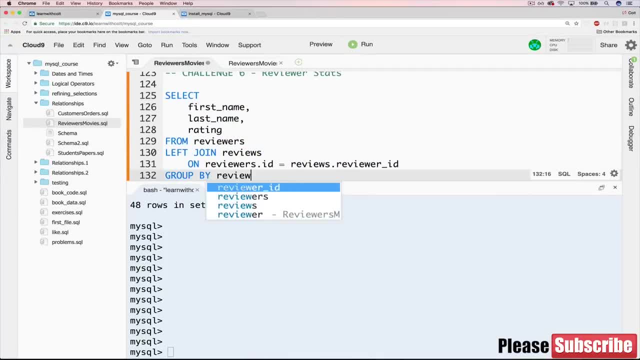 So we can do that now, Group by reviewersid, just like that. And if we do that- whoops didn't mean to expand that. Okay Again, our group by is working its weird magic. It's working behind the scenes. 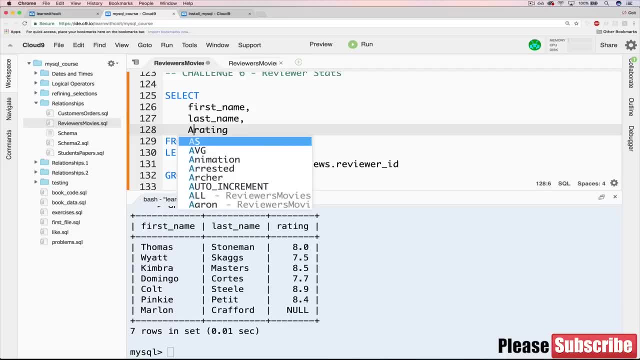 So now we can do things like average, for instance. Let's start there. Well, actually, even easier is count, And we'll just count the ratings. So behind the scenes it's grouped them. Remember it went from this here: 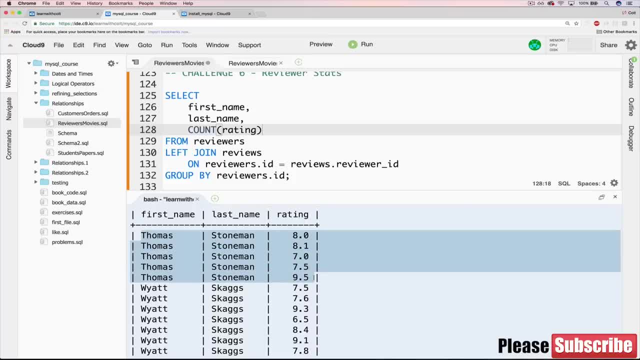 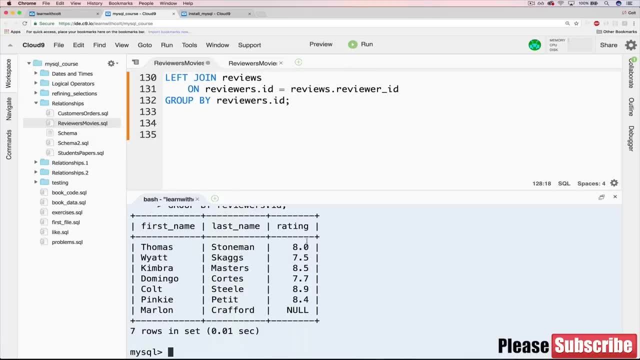 So if we take a look at like these, they were all grouped together. So under Thomas Stoneman there's 1, 2,, 3,, 4,, 5.. But we only see Thomas Stoneman. We don't get five results. but they're there behind the scenes. 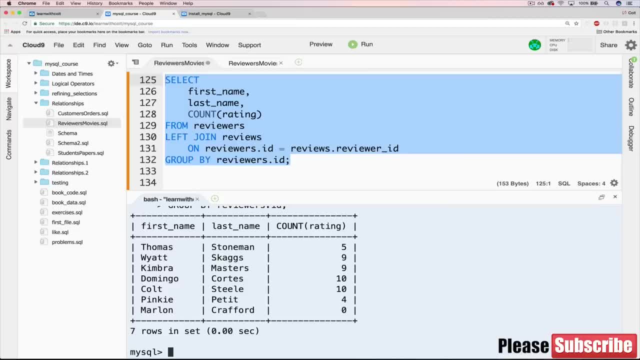 So we'll do count rating And you can see it looks good. We get 5, 9.. You can see Domingo and Colt have written a ton of reviews And poor Marlin just hasn't written any. So that's a start. 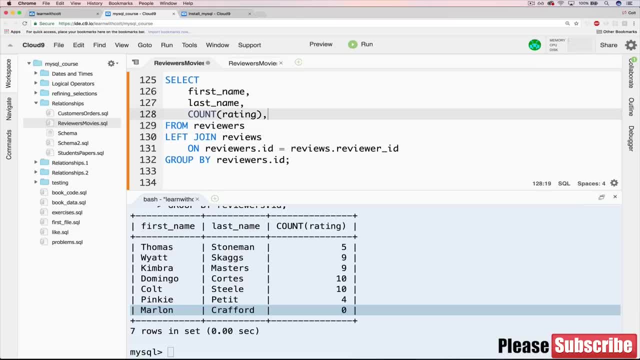 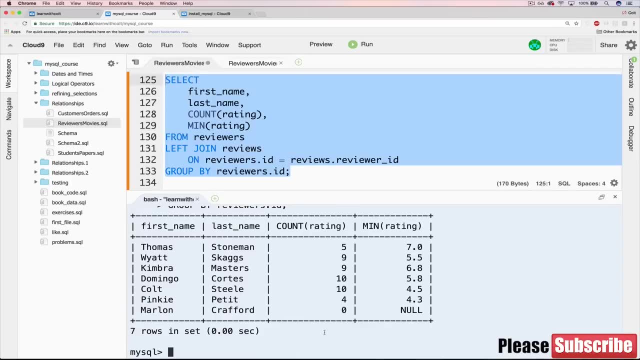 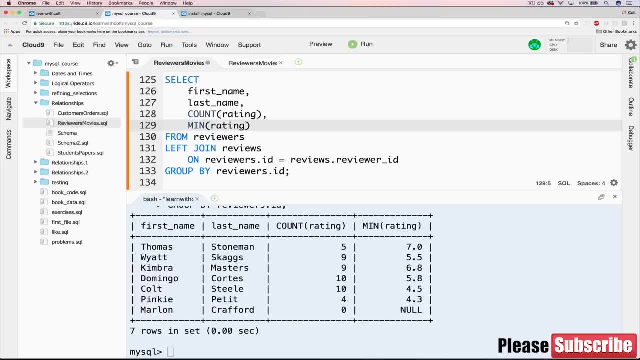 And we should be relatively comfortable with fixing this at this point. Notice that I just sent it to be 0. Could have set it to be anything, You could leave it as null, But let's make it 0 to match the chart. 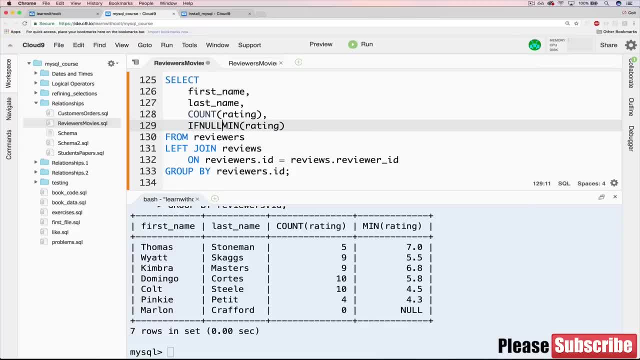 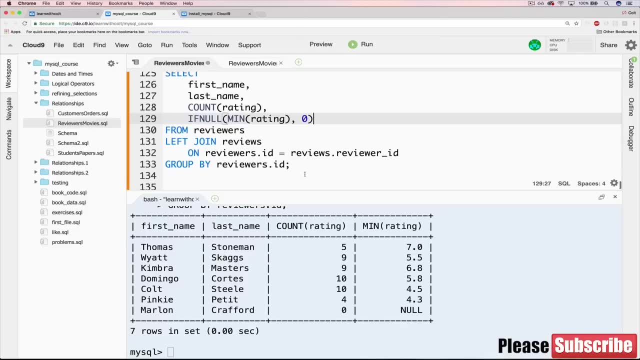 So we can use our if null min rating. Then we'll set it to be 0. And if I leave it like this, our table's going to be kind of ugly because we have this if null up here. We don't need all this space. 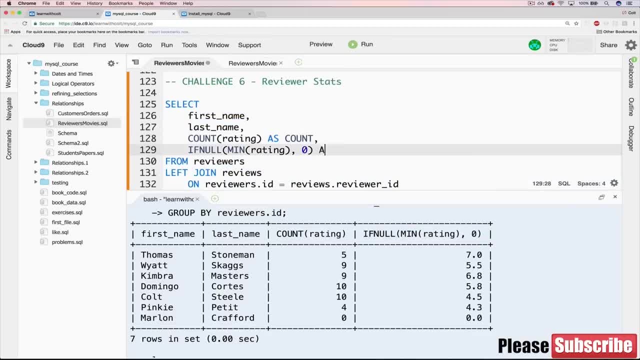 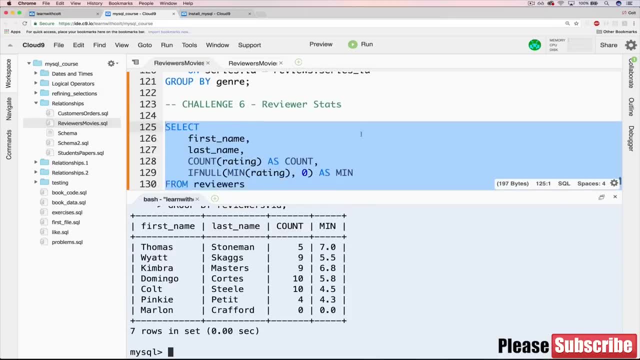 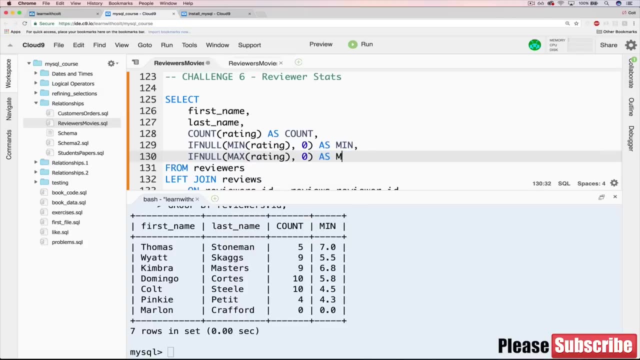 So let's call this one as count and this one as min. That should cut down on the space Looking better. And then the same thing for max, which we can just copy and just change min to max. Okay, So we got min and max. 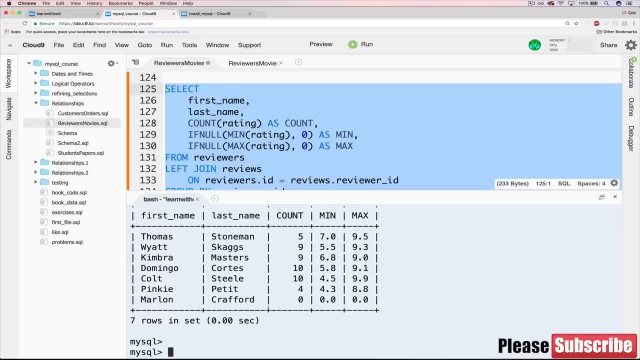 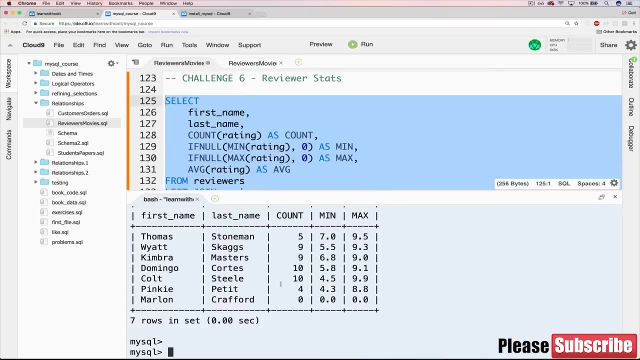 Let's just triple check. There we go, Count min max, Then we've got average, which by now you should be comfortable with doing as well. It's the same thing as average, But we'll run into that same problem with null. 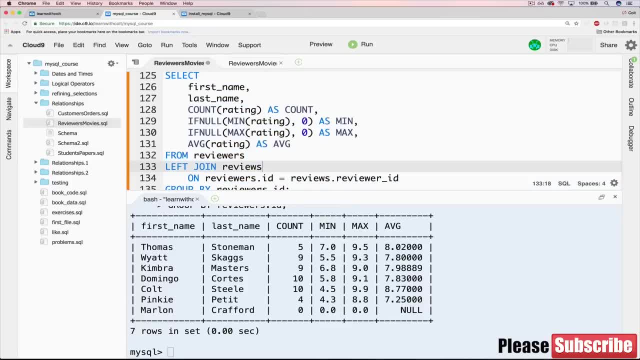 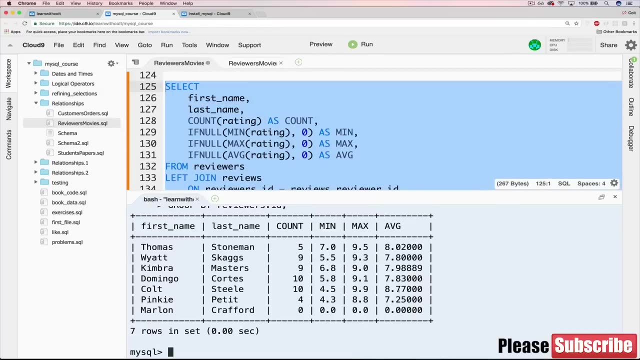 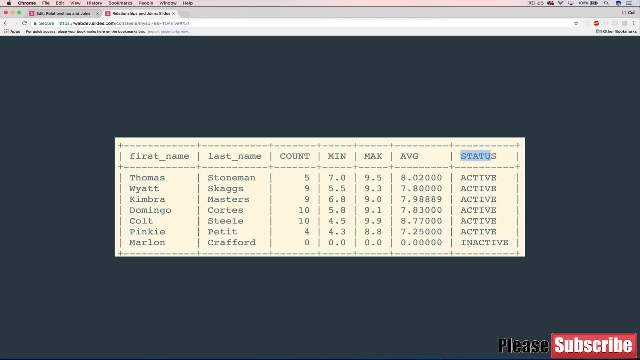 We don't want null there, We just want 0. So if null once again, just like that, We'll copy it. Okay, And we've got first almost everything, except now we need to work with status, And status is a little different because there's some logic here. 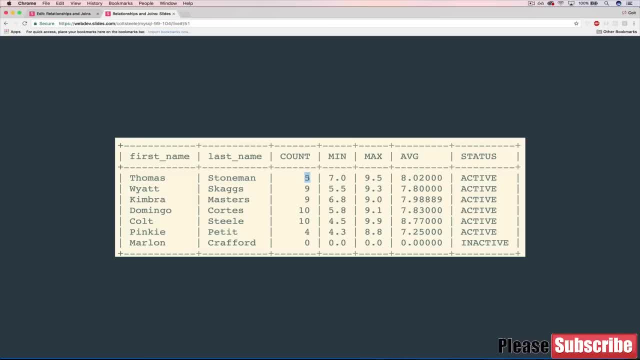 And what's it based off of? Well, it's based off of count. So if count is more than 1, or greater than or equal to 1,, then we'll call that user active or the reviewer active. Otherwise it's inactive. 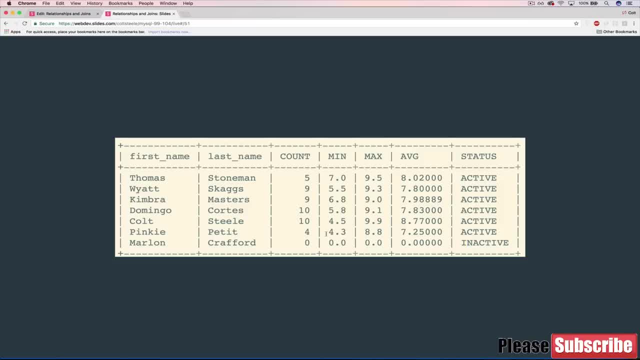 Or we could switch it around. We could switch it around. We could say: if count is equal to exactly 0, then status is inactive. Otherwise they're active. And to do it we could use a case statement. We can start with that. 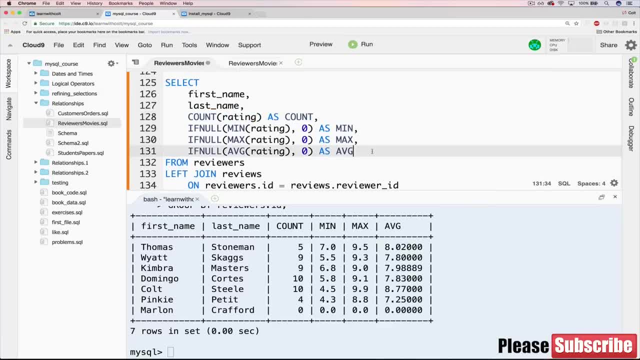 What we're working with again is count, So let's do this at the bottom. our case, And I like to do, end as- and we'll call this status Okay, And our first thing we'll check for in case is when. 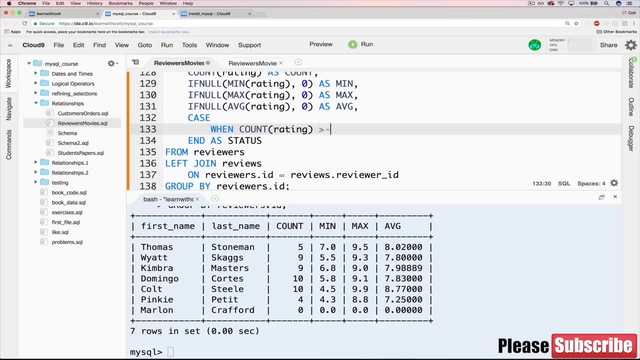 Count rating and we can do when it's greater than or equal to 1, then we'll say active Status will be active Else and we need then here Otherwise inactive, Active inactive. Okay, Let's try that. 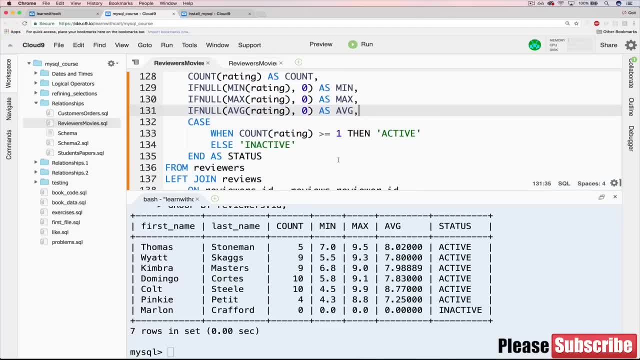 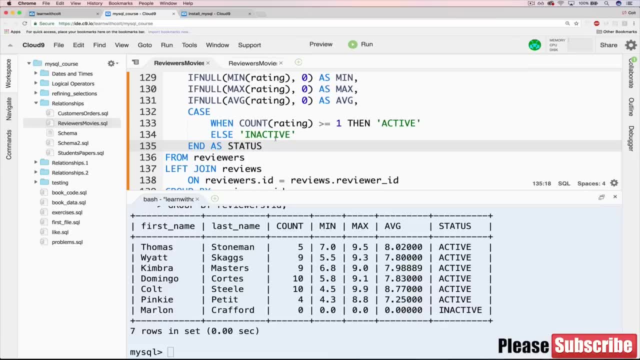 Okay, It works just fine. But I did say there's another thing that we can do, which I also haven't shown you until now. I didn't want to overload you with a bunch of different ways of doing logic. But for simpler case statements we can use another function, another logical function, which is called if. 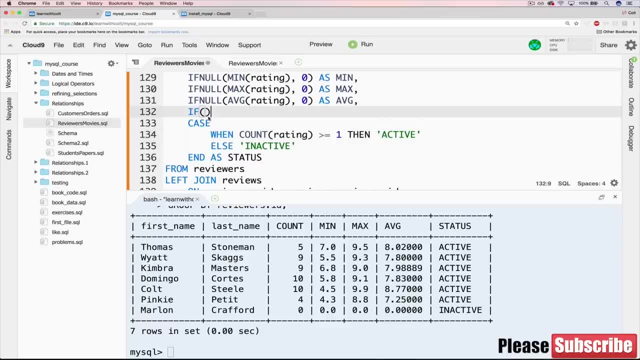 So I'm just going to replace this with if. I'll show you what it looks like. We just say if and then the condition that we're looking for. So if count rating is greater than or equal to 1, then the second argument is what we want. 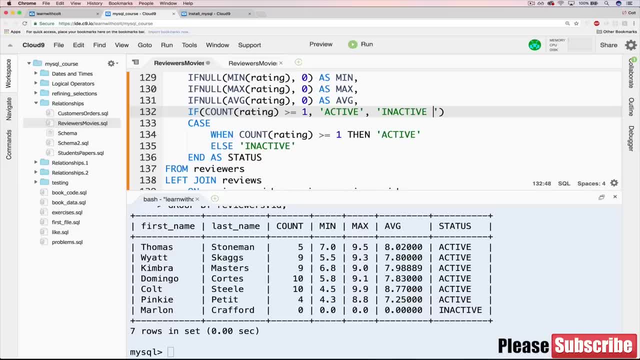 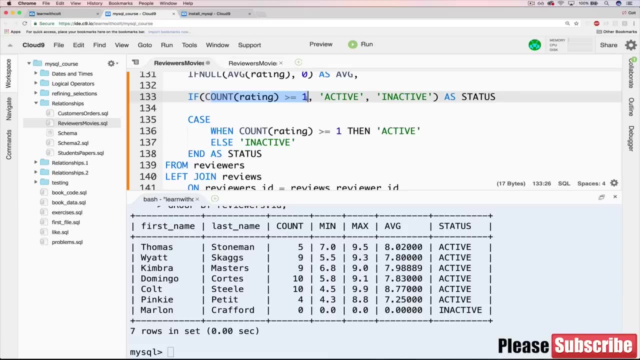 To spit out. And then the third one is the else condition or the else argument. So these are equivalent right here, as long as I put status. So let me make that a little bit easier to see. This right here is saying: okay, if count rating, so if the count of all the ratings per each user or each reviewer is greater than or equal to 1,. 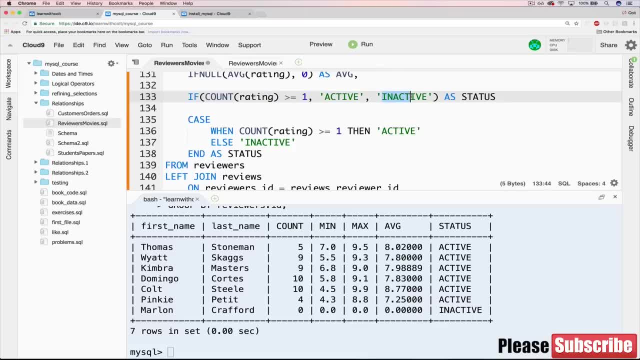 then status is active. If that's not true, status is inactive. So this works. It works great when we only have these two things, that we're working with: right, Active and inactive. But if we wanted to add another thing in, it's a little more complex. 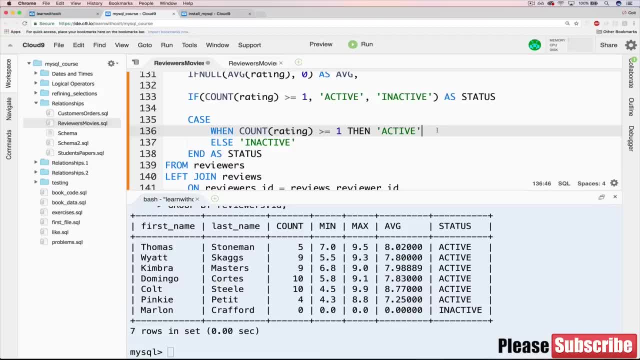 Like if we wanted to say: okay, if it's greater than 1, then they're active, And if it's greater than 10, or greater than or equal to 10, they're a power user or something Otherwise- they're inactive. 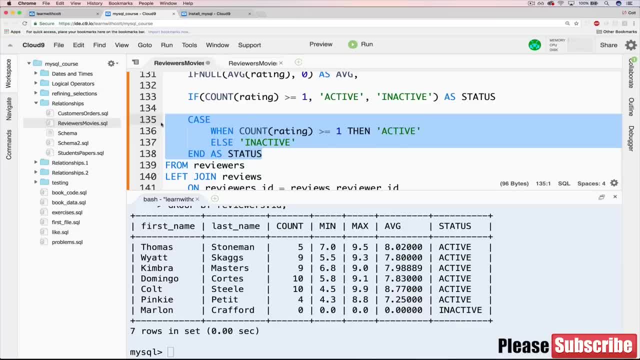 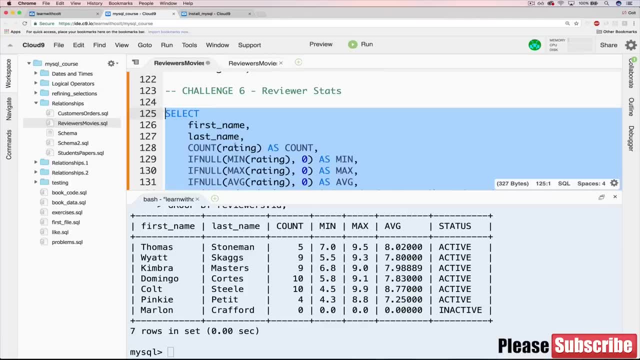 It's much easier to use a case statement for that. So I can show you that. but I'm going to get rid of this first And just make sure that our new addition works The same way. Looks good to me. We could go through and round. average is kind of gross. 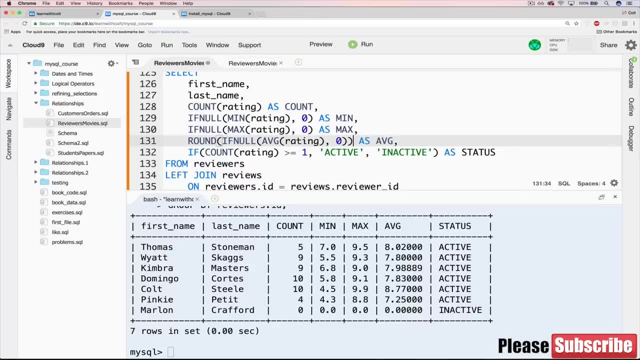 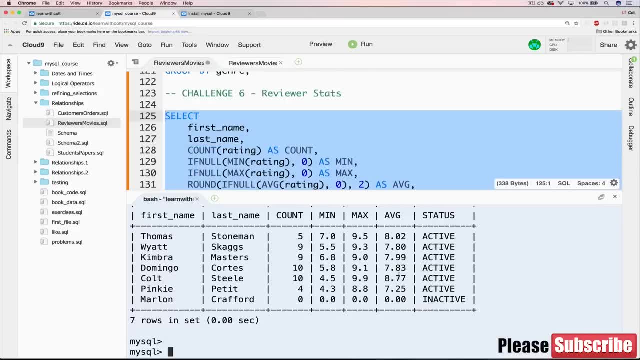 But if we do that, that's going to get quite gross too, And we'll want to break that onto separate lines. We'd want to format that to make it a lot more legible, But otherwise it looks good. So the last thing I'll do is optional. 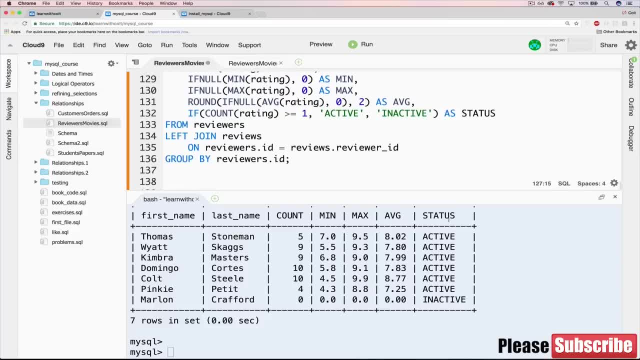 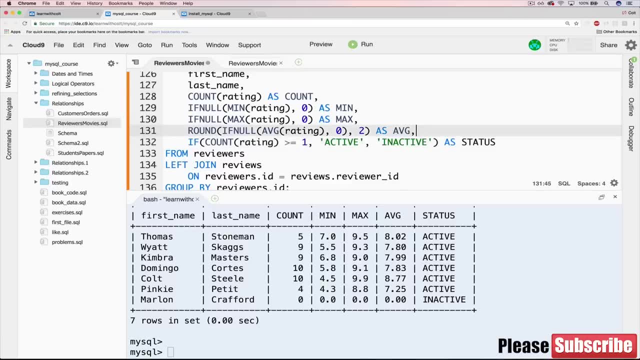 It's just to show you. if we wanted to add in a third status from active, Inactive and crazy active or something like that, we can replace this if go back to our case. So we'll do case and as status And we'll just do case when count rating is greater than or equal to one. 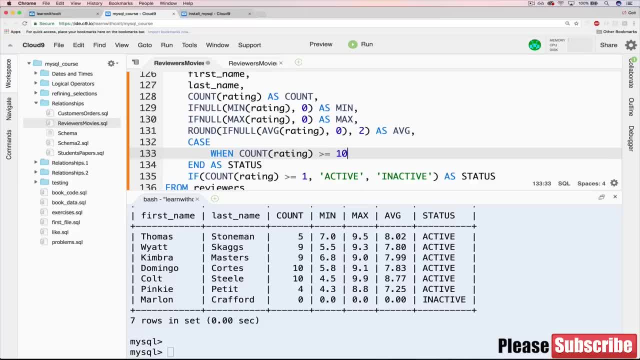 And actually let's start with if it's greater than or equal to 10.. In that case we'll say power user. And then the next thing is: when Count is greater than or equal to zero, We'll just say active. 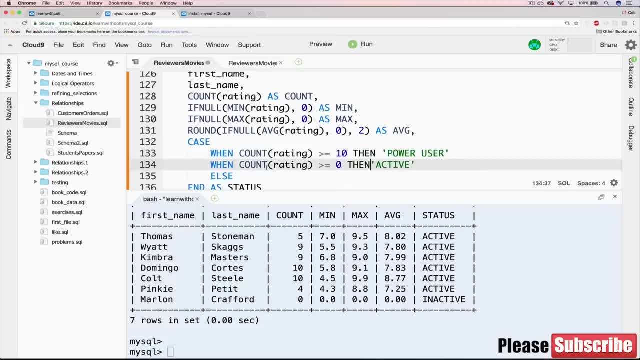 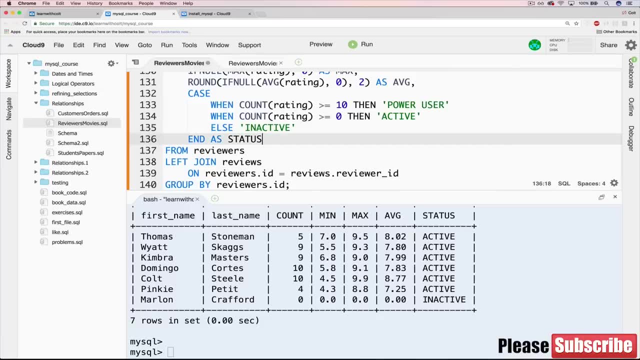 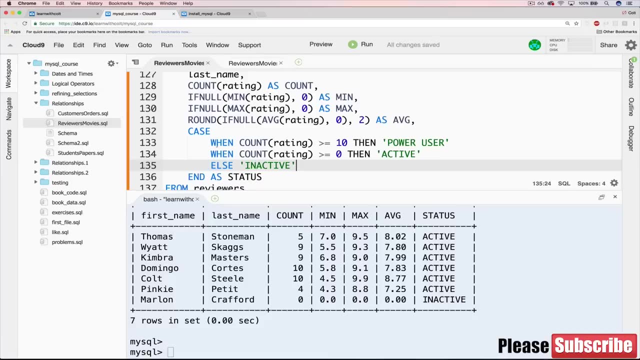 Else, And I need my thens. Always forget those Else inactive. So the way I formatted that is basically to say when. So the way that I formatted that is to say first, Okay, is it greater than or equal to 10?? 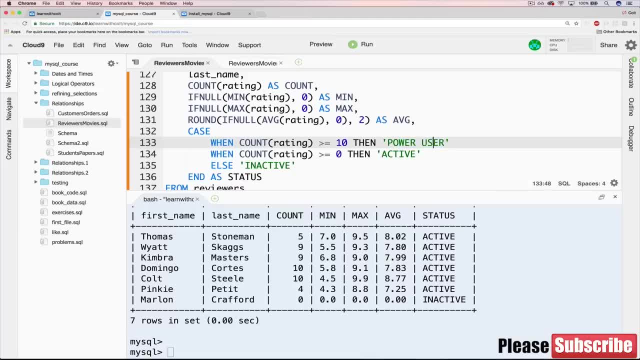 Then it's a power user, Then we're done. But if it's not, that means that it's less than 10.. So if it's less than 10, but still greater than or equal to zero, then they're active. 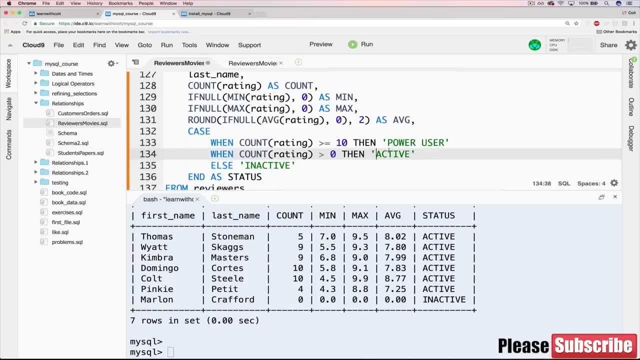 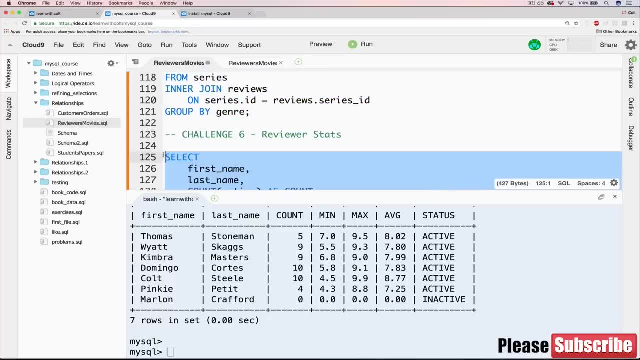 And that should actually be greater than zero, not equal. And then if it's not greater than zero and not greater than or equal to 10, that means they're inactive. So now copy that, paste it over. You can see we have two power users, Domingo and Colt, who have count of 10.. 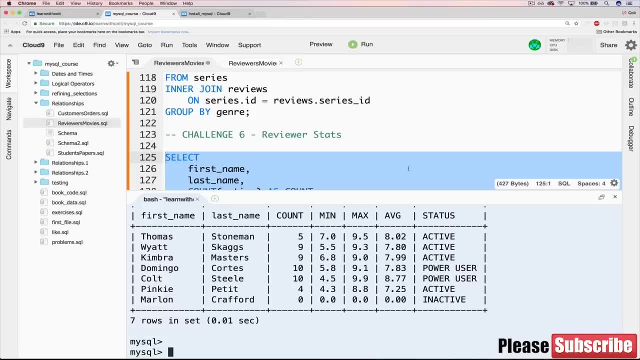 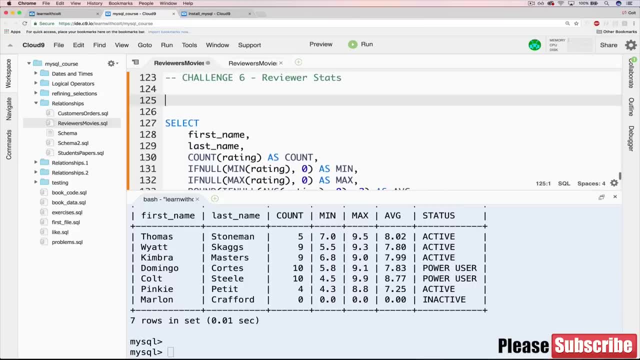 And now we're done. So we made it through that quite a bit there. Okay, Let's go back here. I will leave this example, but I will also duplicate it and go back to having that simple if statement, so we don't have to have the case. 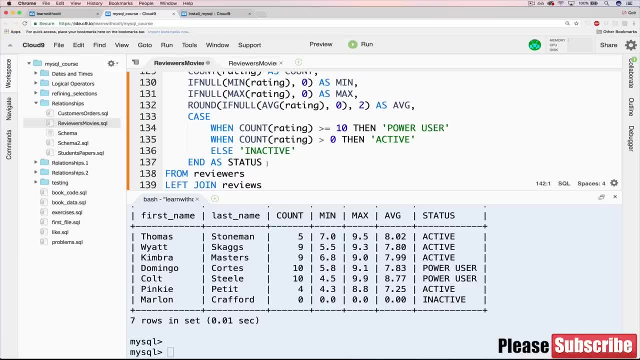 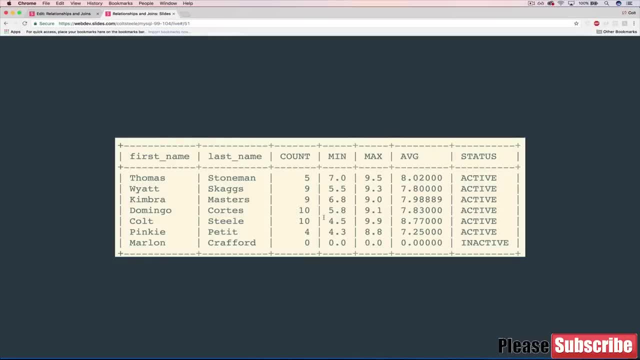 Okay, So I'll do that. You don't have to watch that, But it's in the solution text or the solution file, if you want to take a look. Okay, We're at the final video here, the final challenge, And this is the one that puts everything together, or really more. what it's doing is putting 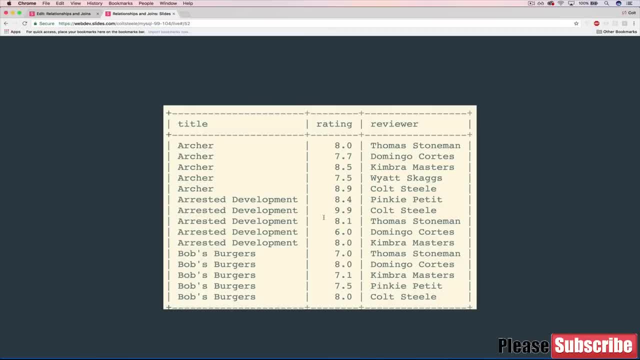 together all three tables that we have. So what we're actually getting out of it is not that impressive, right? We're not doing any crazy analytics or anything like the previous one- Not that that was too crazy, but nothing like that. All that we're doing is putting the title of a movie or of a series and then every. 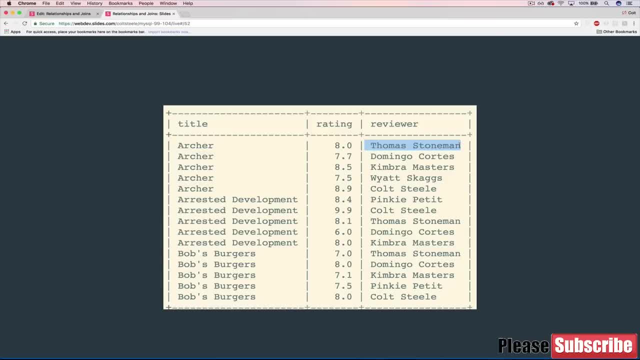 rating that it got along with the reviewer who wrote that rating. So we've done the first part up until here, right where we've done title and rating together, or where we've done reviewer and rating together. But now we're going to put them all together so that this is the information for one review. 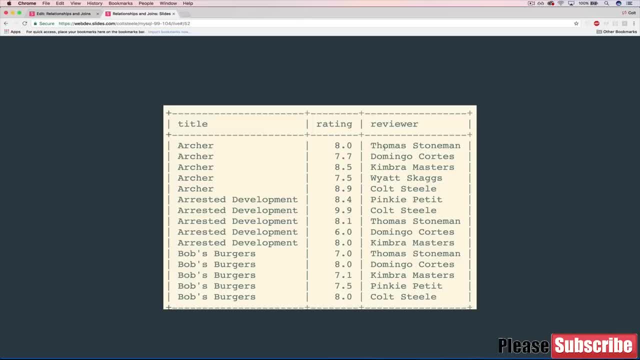 right, It's the movie that was, or the series that was, reviewed. It was the person who reviewed it. Notice that we can cat them into one reviewer instead of first name and last name, but that's secondary at the end. So we have the series title, the reviewer's name and then the rating they gave it. 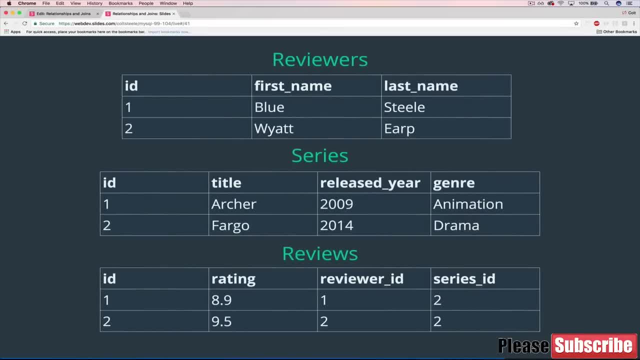 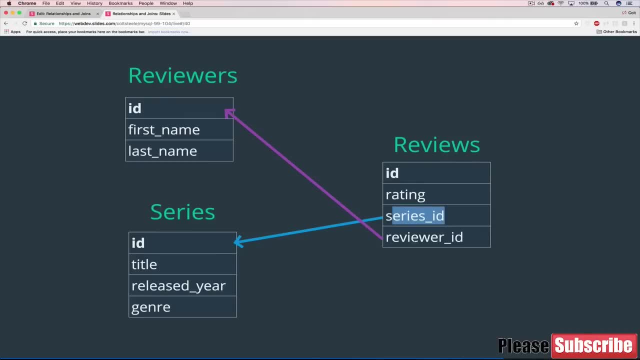 So we're basically just trying to take- let's do it here- take this and fill in the blanks. So, instead of series ID, we're going to get the name of the series. Instead of the reviewer ID, we're going to get the name of the reviewer. 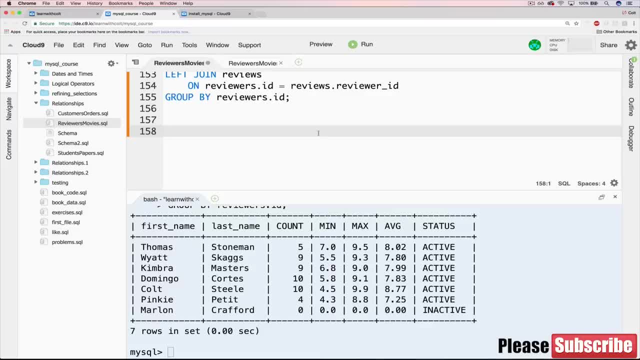 Okay. So let's go ahead and start over here with our handy dandy comment. And we are on. what is this? seven, six, yes, seven, three tables, Okay. So we can start off with any of the tables. 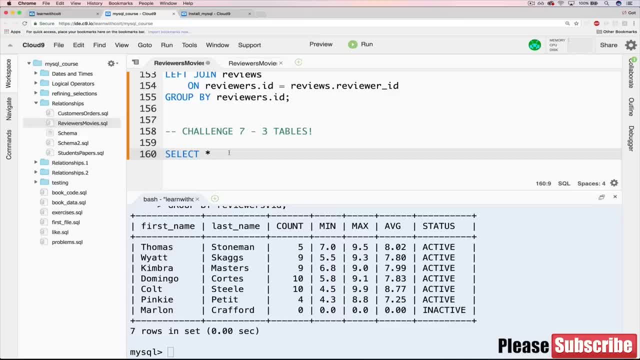 We're going to join them all together. Okay, So I'll start with reviewers. So we'll select star from reviewers, just like that. except I need from boring. We've done this before. blah, blah, blah, blah blah. 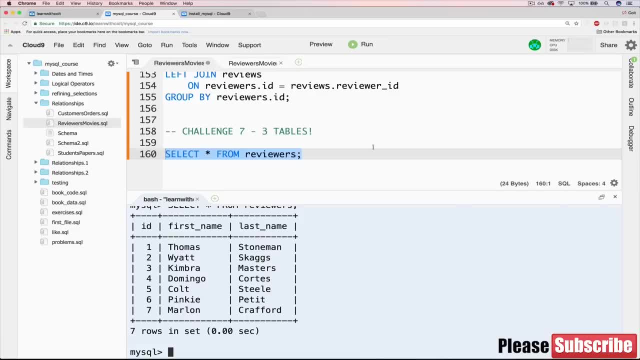 So the first step is to join it with the reviews table. So we'll have review ers along with their reviews, along with the series associated with that review, And we're not going to worry about, You know, people who haven't written reviews. 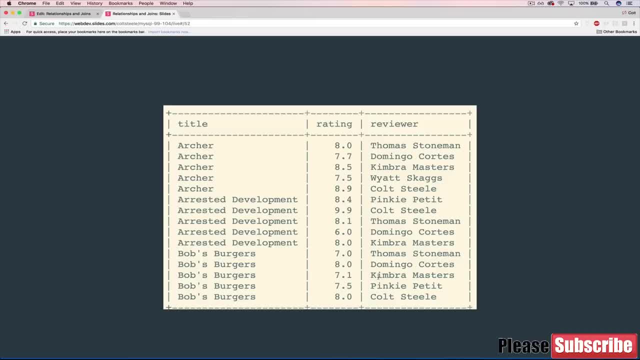 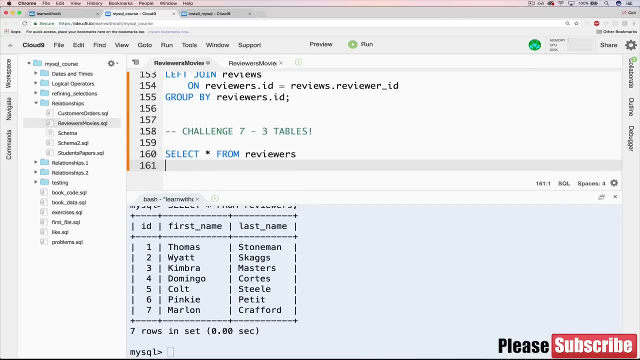 That's fine. We're ignoring that, Okay. So to do this, let's start off first of all by joining it with join reviews on reviewersid equals reviews dot. and then we need reviewer ID- So fun to write, And we do that. 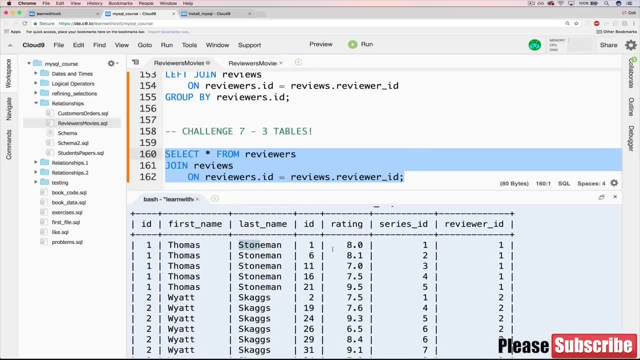 And we see things like: okay, Thomas Stoneman gave an 8.0 to some movie, that there are some series with ID of one. He also gave an 8.1 to whatever has ID two, and so on. So we're getting close ish. 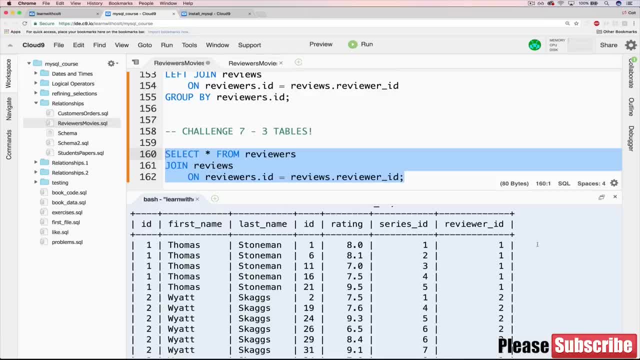 Now what we need to do is also throw on the series data over here, And the first thing I'll do is just make this explicit: It's an inner join, So we're going to do another join and it's really easy. At least syntactically it's easy. 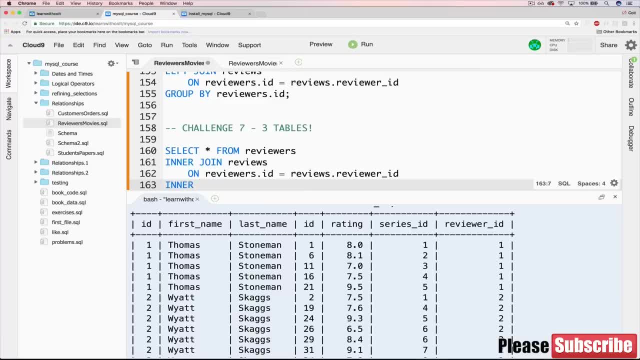 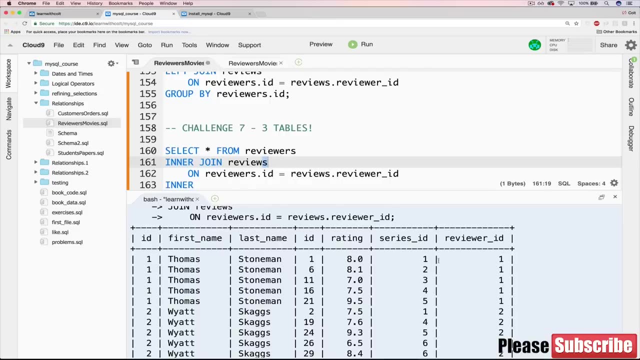 We just write inner: join again. So what are we joining on this time? Well, we're now going to join on the only thing that's left, which is series. So we took reviewers and reviews, sandwich them together where they intersect. Now what we're going to do is join a series where the series ID is equal to series ID. 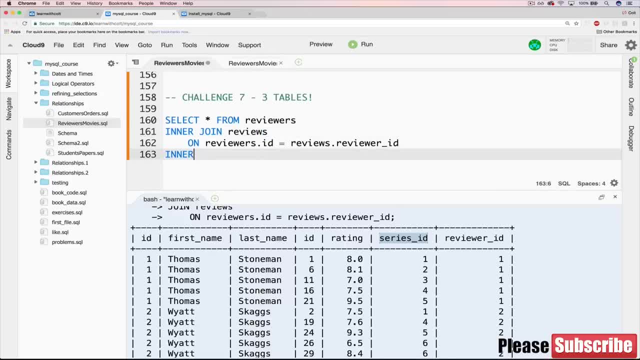 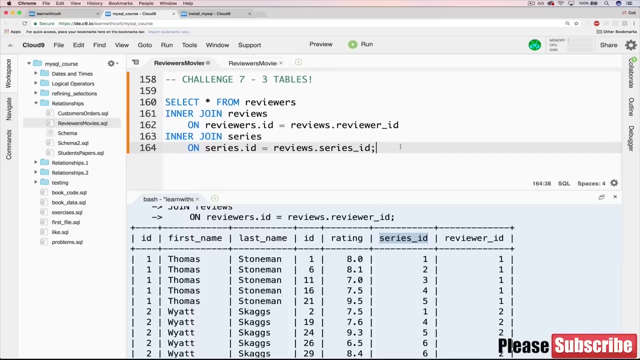 here inside of the reviews. So let's do inner join series. Reviews on series. dot ID equals reviews. dot review or dot series underscore ID. Such a nightmare trying to speak all this out loud, But let's step through this. Okay, so we have sort of this middle table. let's say which is right here. 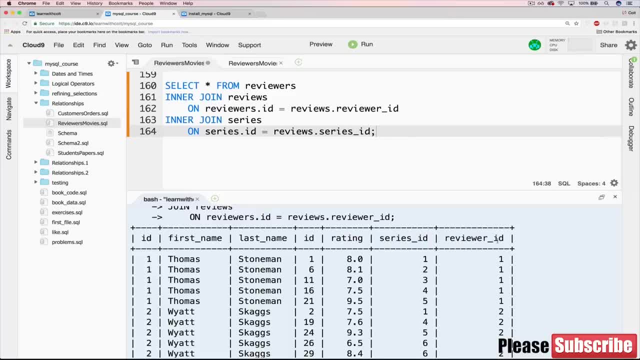 We have ID, rating and Series ID and reviewer ID for our review. That's, every review has that, And what we started off was joining it with the relevant reviewers. Now we're going to also take the series ID and find all matching series and stick them over here. 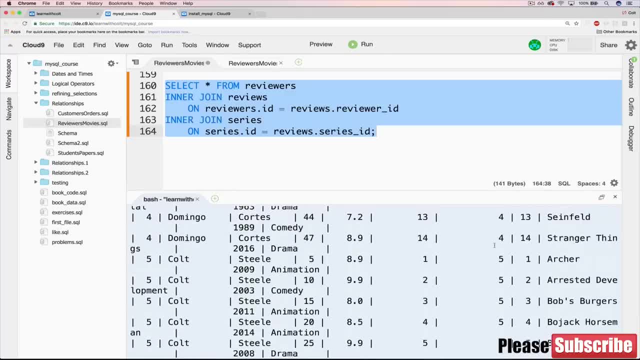 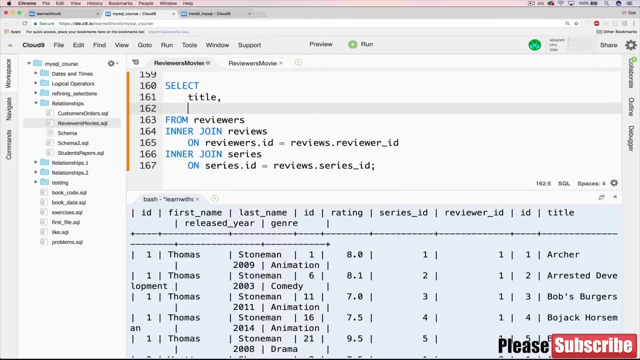 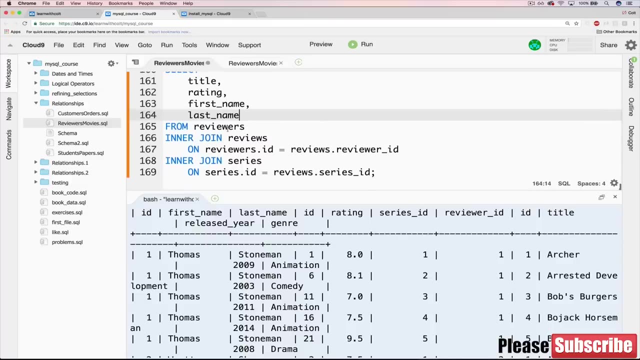 And it's going to be a messy table. It's going to get all collapsed and screwed up. So let's filter out some things. So let's only work with the title, the rating, first name and last name. Okay, so we're getting close now. 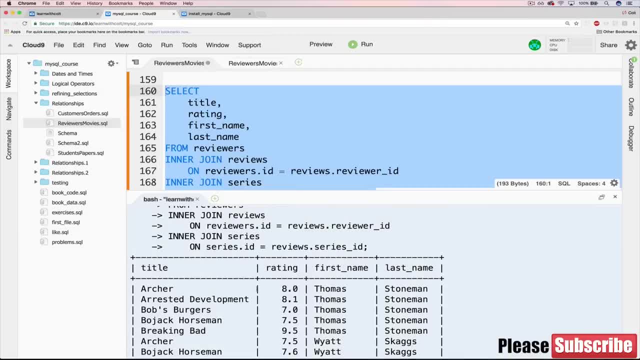 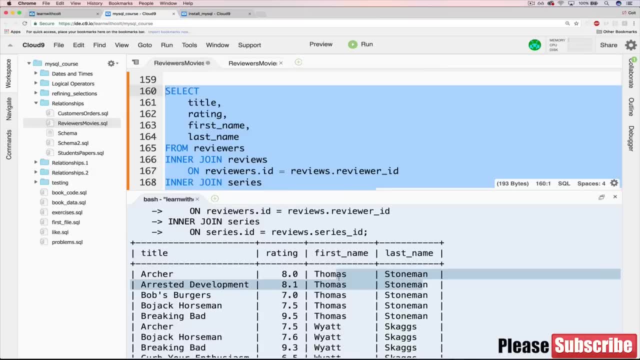 So we're pretty much there. We have all of the data together. So we have: Archer has an 8.0 rating from Thomas Stoneman. Thomas Stoneman also gave Arrested Development an 8.1. And he gave Bob's Burgers a 7.0.. 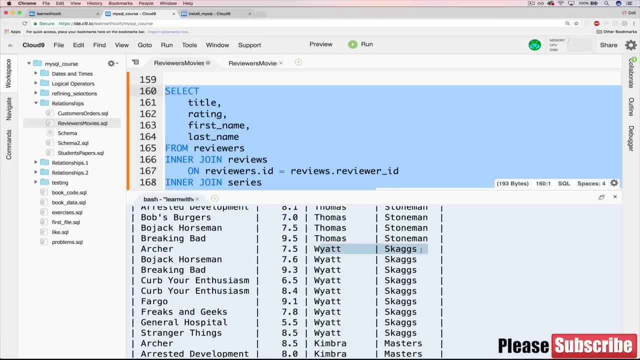 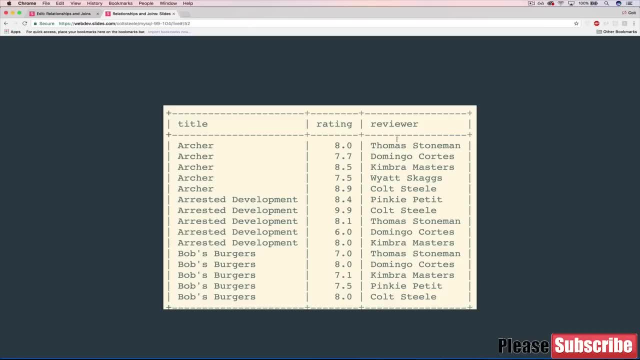 And then we can see: okay, we have Archer again down here from Wyatt Skaggs, who gave it a 7.5. So we have all of our data synthesized in one table. Now what we need to do is concatenate things together over here. 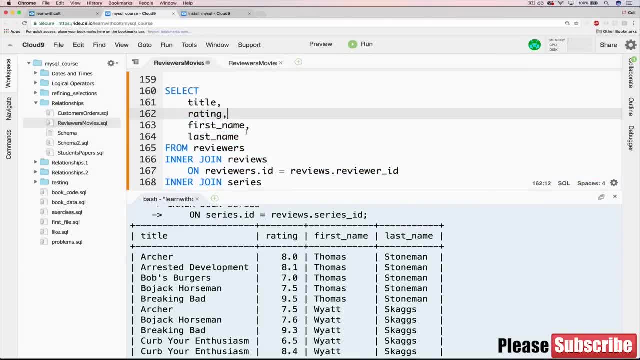 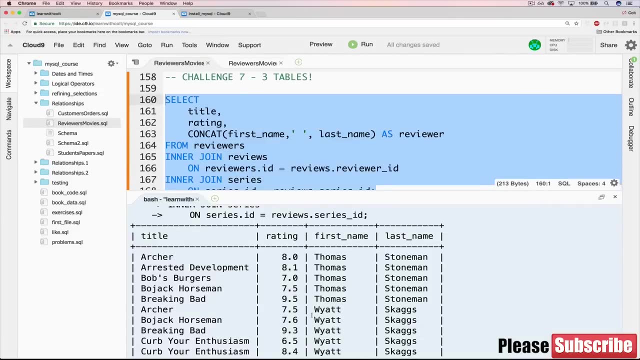 So that's just simple. All we need to do is, instead of doing first name and last name, we'll do a concat: first name, comma space. last name as reviewer, I think is what we called it- Yep, Okay, And then there's only one thing that we need to change, other than that which is right now. things are ordered by reviewer. 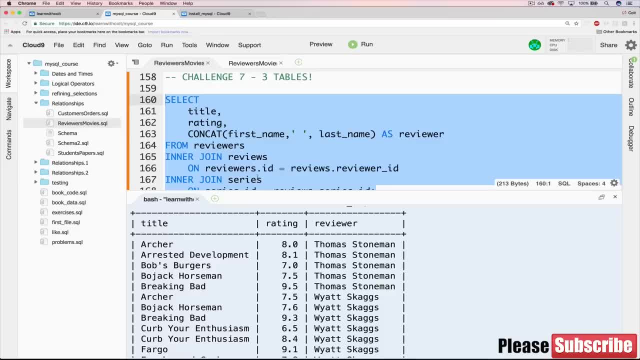 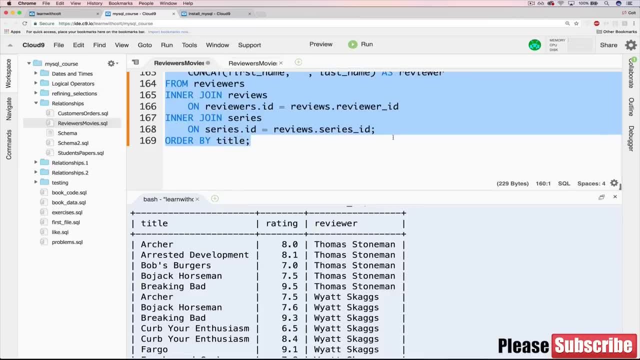 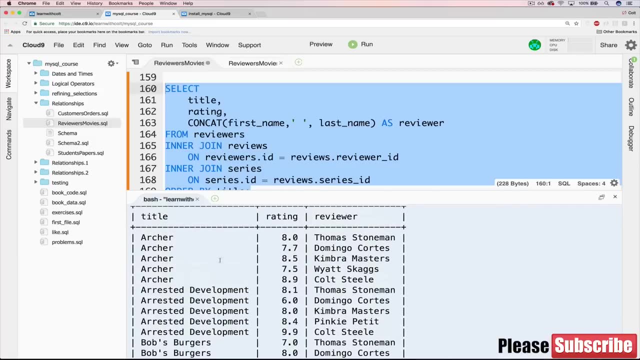 Let's order them by title, which is what we did over here. So that's just a simple order by title. Now we should be done, If I get rid of that extra semicolon, And here we go. So we have Archer- all of the ratings for Archer and the people who wrote them. 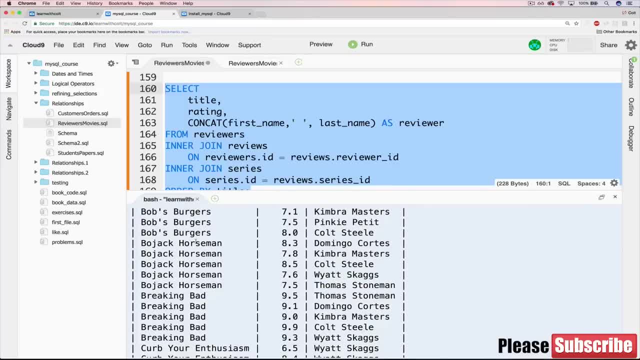 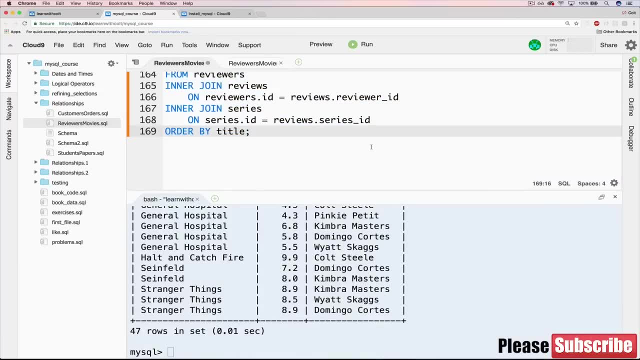 Arrested Development, all the ratings and people who wrote them, And all the way down through all of our series that have reviews. So that's important. It's only where we have reviews. So to summarize, let's go all the way back here. 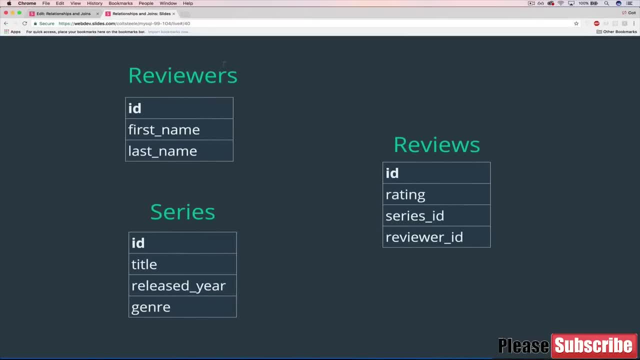 What we just did was basically take the reviewers table, smash it with the reviews table where they match. It's an inner join where the overlap right. So we take the overlap between them based off of ID here and reviewer ID. Then we have that second table that we then joined with series, where the series ID matched the ID of a series. 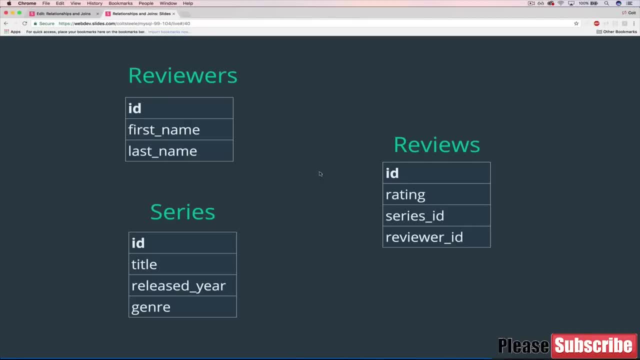 So it's a three way: two joint statements but three tables together, And that's why I decided to do many to many relationships after the simpler one to many, But hopefully it's not too intimidating. We did a bunch of exercises with them. 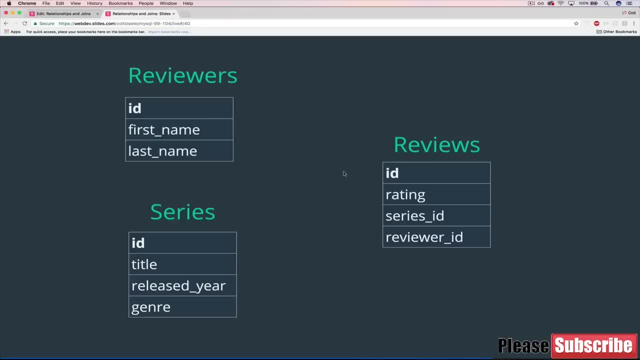 You're probably a bit burnt out- I know I am from recording all of them, So I definitely recommend that you take a break before we move on. We're going to continue, of course, with joins and relationships, But we're only building from here on out. 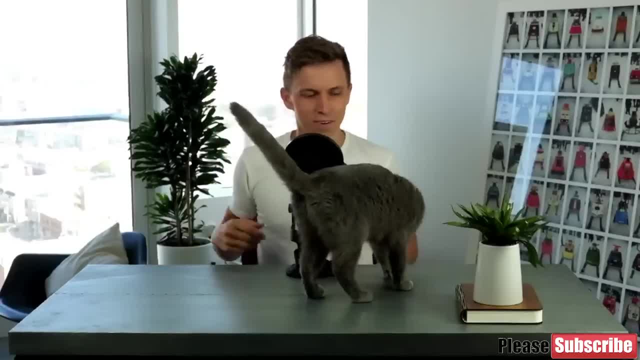 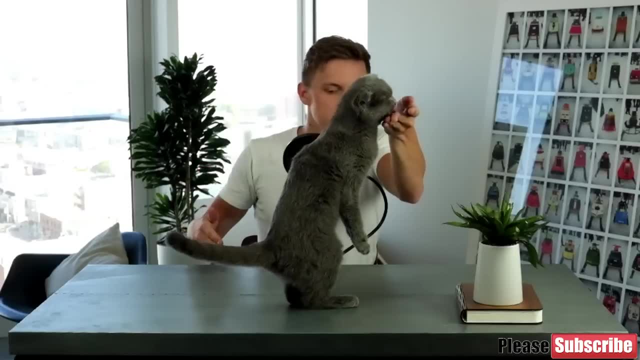 So congrats on making it through This part. Hey, welcome. I'd like to show a couple of things. Here's a nice trick blue can do. Look at that, She's like a, like a T-Rex or something. Great job. 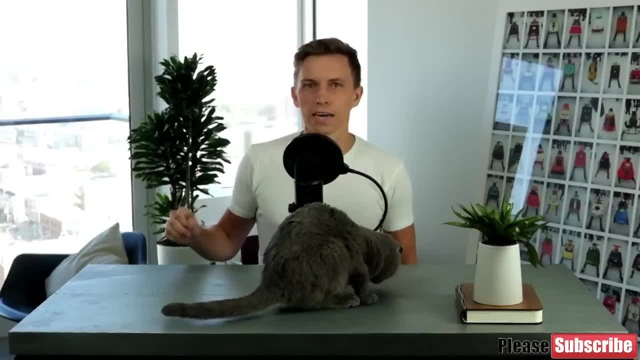 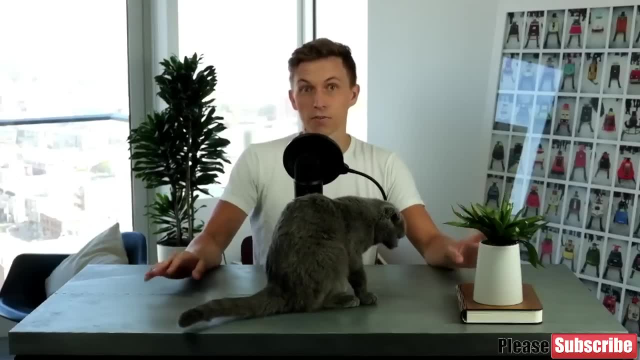 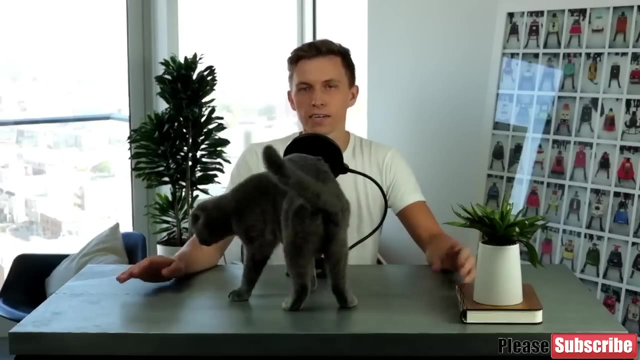 That's the first thing, But the second important news that I have here is that this section is the one where we finally do our Instagram data, or are finally cloning Instagram, And that's actually an exaggeration. We're only cloning the database, And even then we're only doing like seven or eight tables, not, you know, 20 or 50. 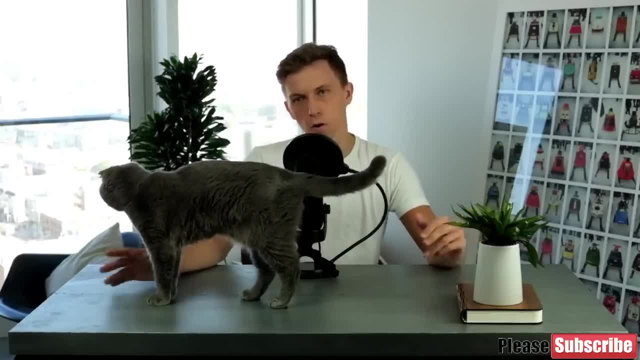 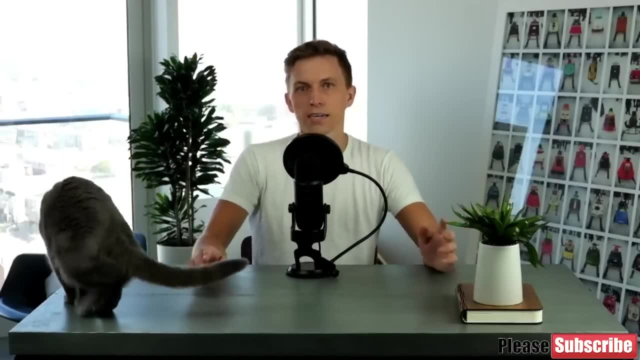 Instagram tables, But still we're doing the basics, the important stuff: photos and comments and users and likes and follow. you know, follower, following, relationships, hashtags, all that fun stuff, all the relationships between them And then all those joints. 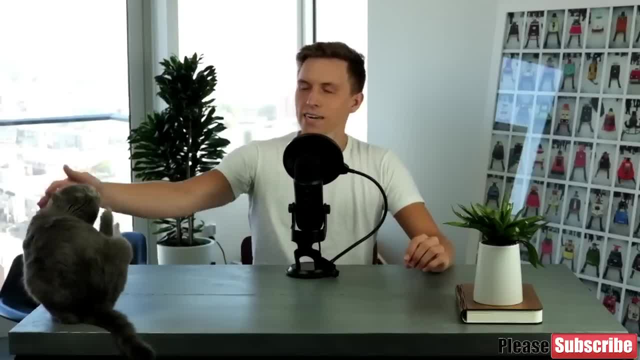 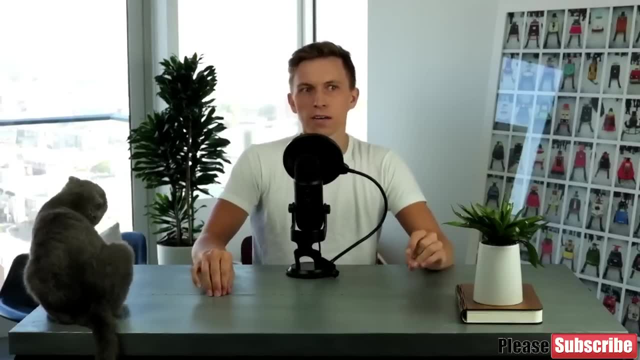 There's a lot of opportunities there. So this is sort of acting as a bit of a end cap on this course. It's not the end, but this is the last kind of data set that we're working with, And then I'm going to show you after this. 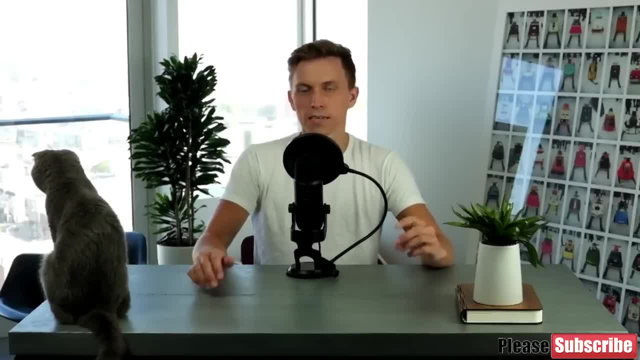 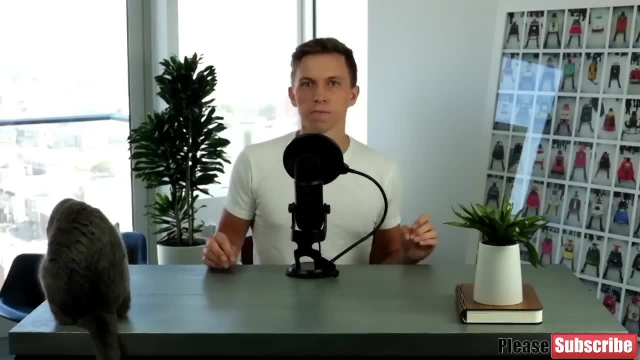 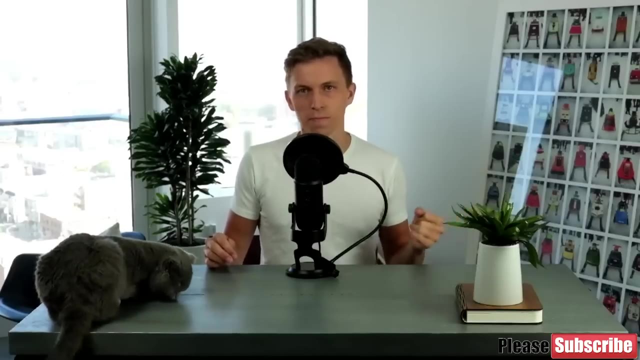 How to build a Web app with MySQL. So that's also coming up, which hopefully is exciting. But this section, like I said, is all about Instagram data- really exciting stuff- Going to basically build the schema And then the next section is going to be a bunch of challenges and problems with it. 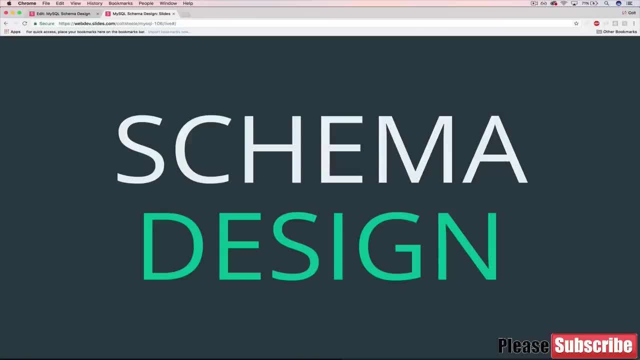 OK, let's get started. Hello, welcome back. So this section is going to be a bit of a capstone- Maybe that's an exaggeration. It's going to be a summary of what we've been focusing on in the last couple of sections. 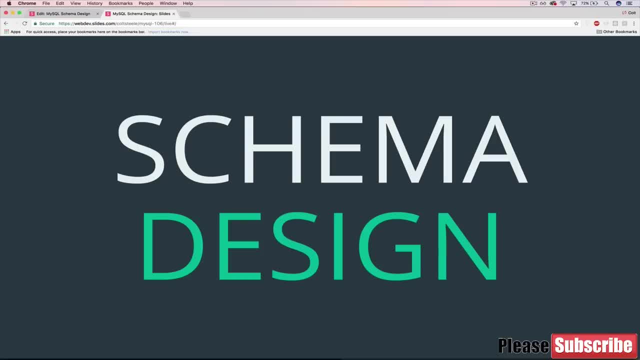 So there's sort of this subsection of the course, the last three or four sections- that we're all focused on working with multiple tables, relationships between data, tables where we have foreign keys referencing other tables, talking about relationships or associations like a one to many relationship or many to many. 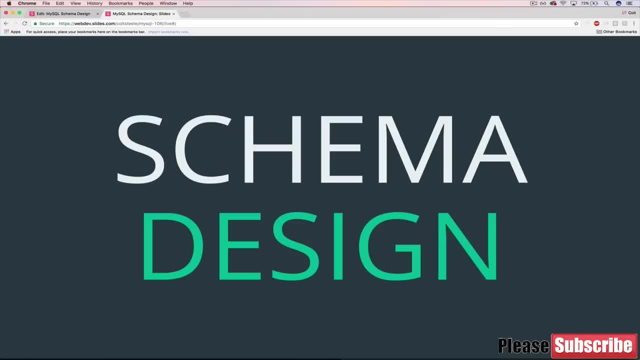 relationship and so on, and then also joins, which is what we are focusing on as of late. So this is going to kind of wrap that all together Into something bigger, because so far we've really been working with two, maybe three tables, modeling a single relationship like customers and orders. 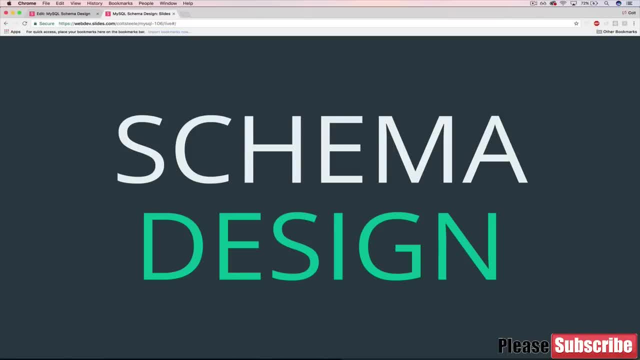 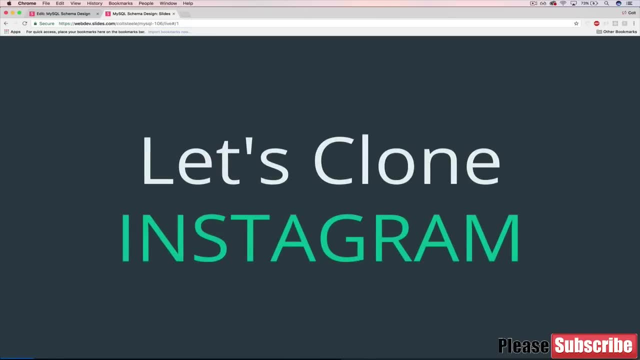 But now we're going to take something on a little bit bigger. We're going to focus on a bit of a case study. We're going to work with a site that you're probably familiar with- Instagram- and we're going to try and clone the database for some of the basic functionality. 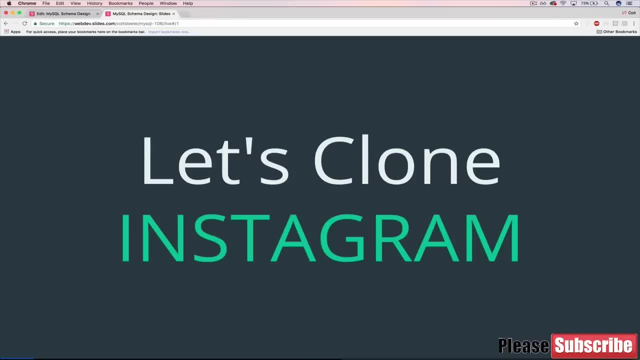 So we're not going to be diving into like using and keeping track of our users data and all of that. We're really focusing on the main big entities to a site like Instagram, things like photos and comments and users and so on. So again, we're not really scratching. 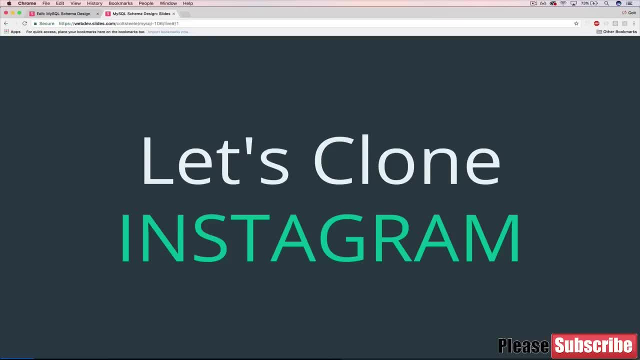 the surface as to how Instagram actually stores everything. We'll talk about what things work best for scaling. We'll run into some fun issues when we talk about how hashtags work and how you should store hashtags, So we will talk a little bit about performance. 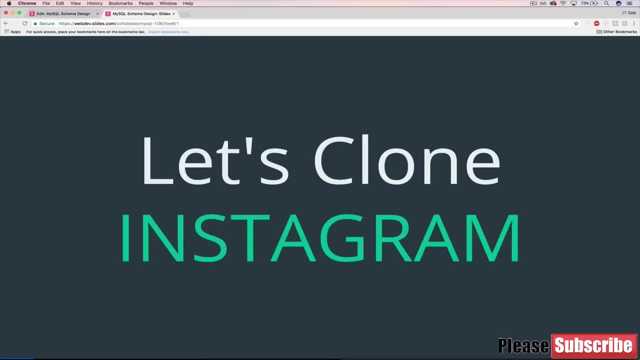 But this is really more about how do you create a schema for something that has, in our example, at least seven or eight tables. In Instagram, the real app, there's probably dozens of tables, But either way, it's a big step up from two tables or three tables max. 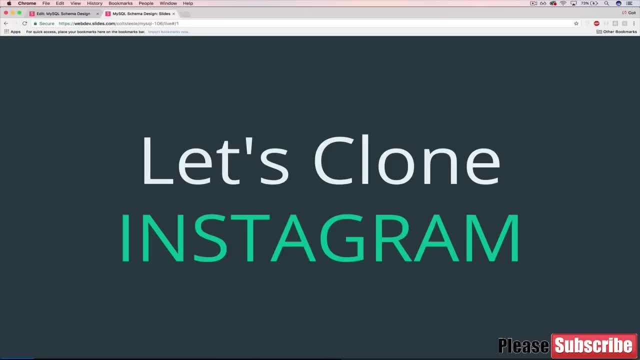 And then the other thing I want to mention is that in this section we're going to focus on designing the schema. It's going to be a bit of an exercise, but I'm also going to go through and do it myself. But then in the next section I'm actually going to give you a bunch of data, like a ton of data. 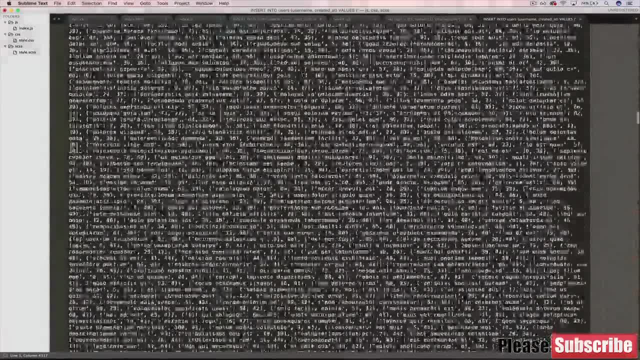 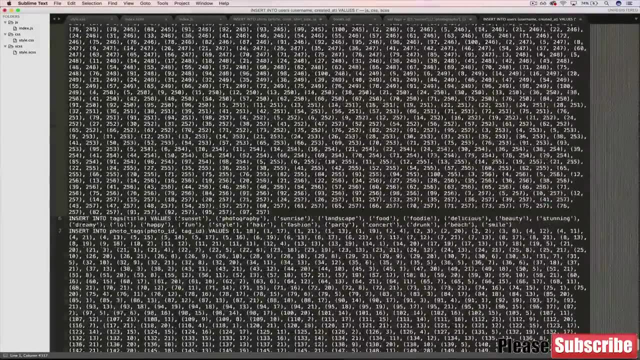 I spent a long time making this here, So this is what we'll be working with. You'll actually be inserting this so that, for once, we'll be able to work with big amounts of data, thousands of rows, and you'll see the impact that it has. 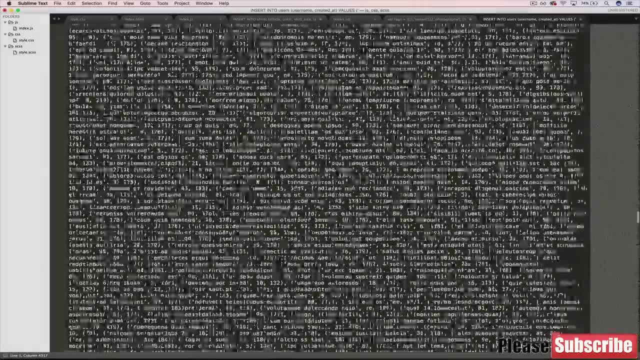 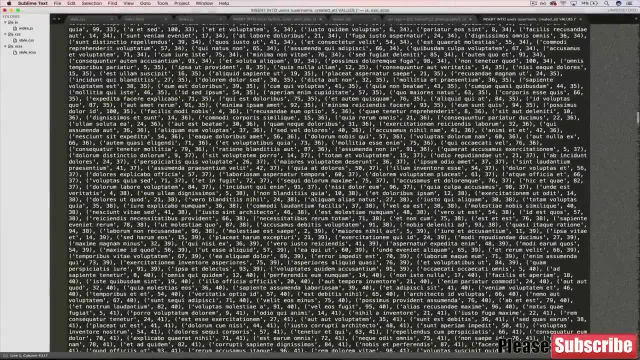 And also, hopefully, it will feel a bit more realistic rather than two or three things at a time. So that's where we're going, But in this section we got to create the schema first. We got to understand what we need. So let's start by taking a look at typical Instagram page. 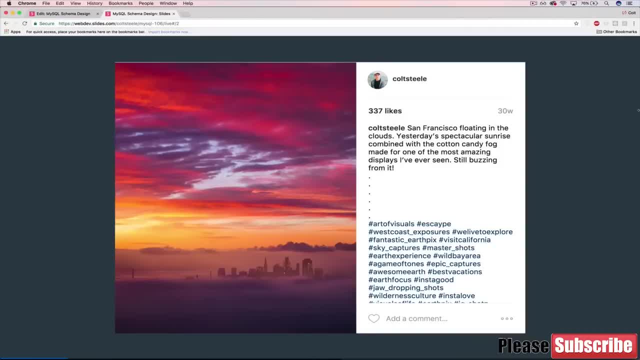 And yeah, some of you may know this, I'm in my spare time. I like to do photography, especially landscape photography stuff around San Francisco, So I am using my own Instagram here, but that's not really why I'm not trying to get more exposure or anything. it's just that I don't want to run into any. 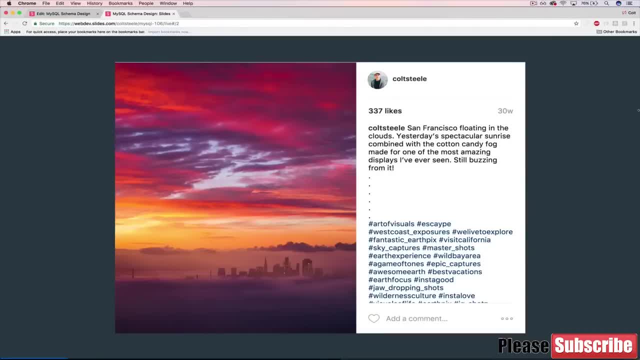 issues with permission or using or having rights to use somebody's images in my course, OK. so, with that said, the reason this is here, like I said, it's not just to show you my photo, but mainly it's to help us understand and identify the key entities. 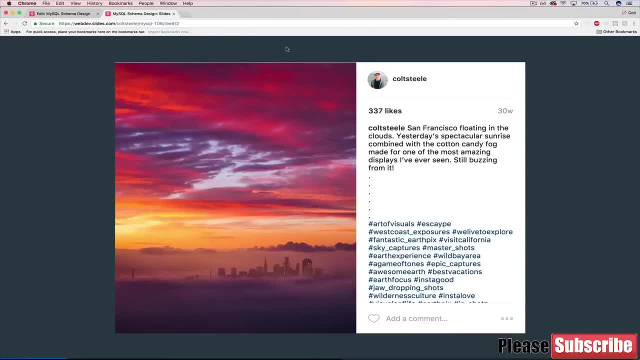 So, on this basic Instagram, this is from the web app, though most people use the iOS or Android app. It's the same entities, the same data, And the first thing, probably the most obvious, is users. So we're going to need some sort of users table or a way to store users. 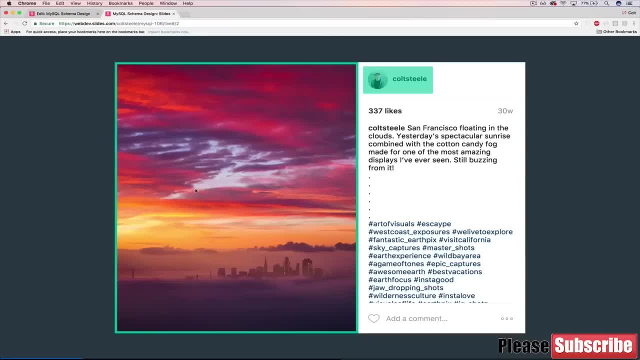 And then, moving on, we've got a really obvious one, which are the photos. We need a way of storing images or photos. Now, we're not going to worry about how we actually upload photos and how, what data type we use to store them or anything like that. 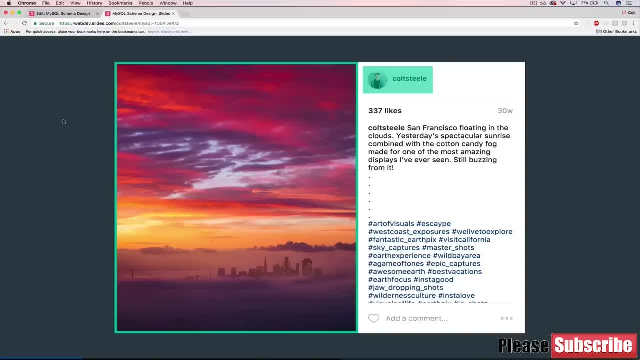 We'll just say that it's an image URL. So when we actually get to the exercise portion, I'll come back to that. So we need to store stuff about photos. and then we've got things like likes. So we need to store likes for a given photo. 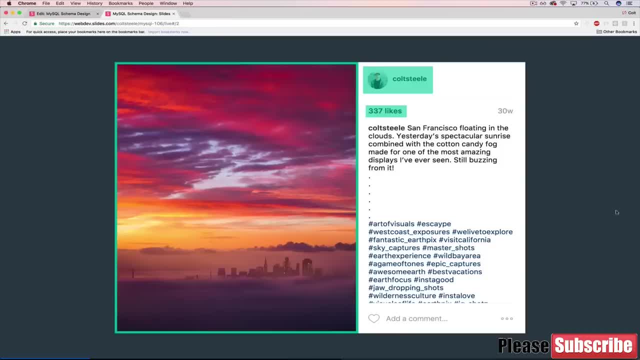 But also remember there are some complications because I can't just click on this heart button ten times and add ten likes. I can only like it once, So we need to have something there as well. Maybe there's something we can do with our database. 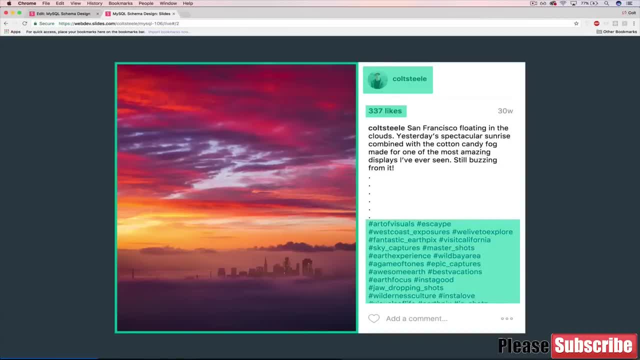 And And. then we've got hashtags, and hashtags are fun one. We're going to save that for last in this section, because there's a lot of ways of doing them. We'll talk about at least three, And there's a couple of advantages and disadvantages to each. 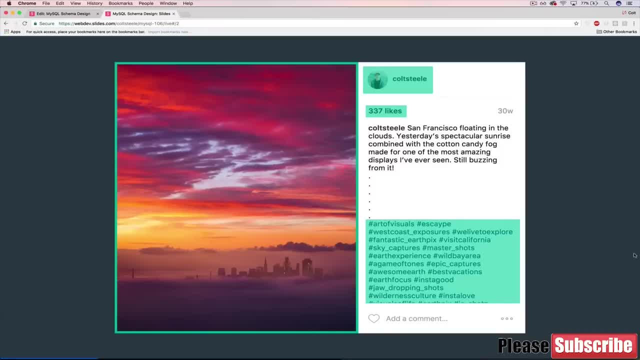 So hashtags, though, are important. Part of Instagram and of a lot of tagging in general, is a lot of Web apps, whether it's blogging or Twitter or something like Instagram, And then we also have other components that I couldn't fit onto one page. 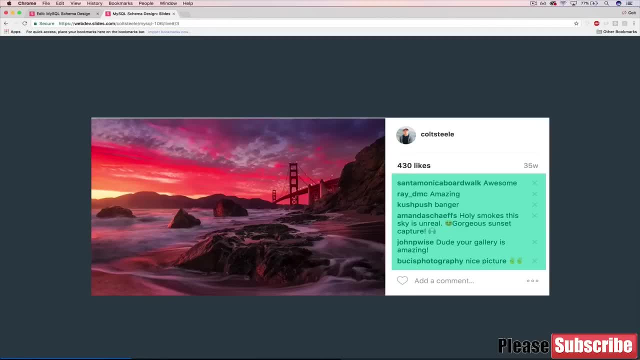 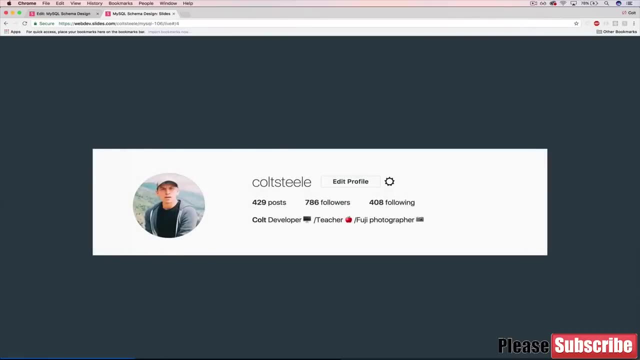 So, like comments here, that's really the big thing that we also need to be able to store comment information. And then there's one other big thing, which is followers and following, So the relationships between users. How do we store that? You know, there's a couple of ways of doing that as well. 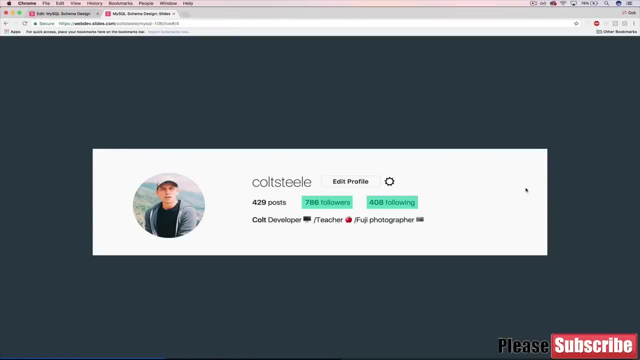 But on Instagram, the way that it works and the way that our database should work is that it's a one way relationship. It's not like Facebook, where I send a request to someone and we can only become friends if they accept, or vice versa. 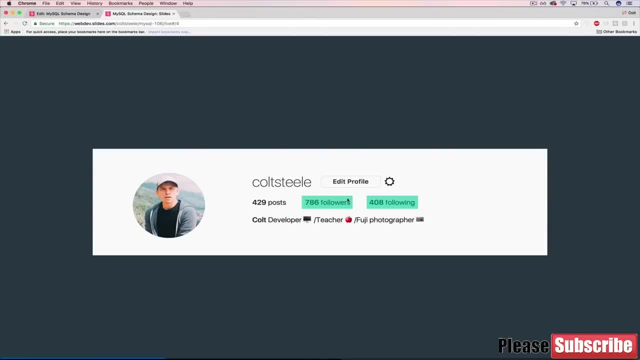 But both of us have to be kind of consenting friends. on Instagram, I can follow somebody and they don't have to follow me back, or people can follow me and I don't have to follow them back. So how do we store that in a database? 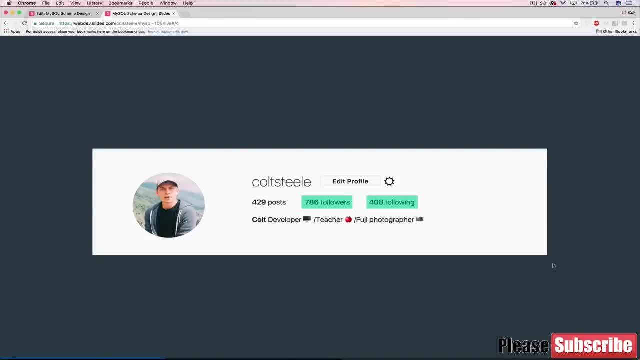 OK, so that's really what we're focusing on. There are obviously other things, like we're not going to store profile information, We're not going to store stuff about advertising, like I said, and that's just scratching the surface of what we're not storing. 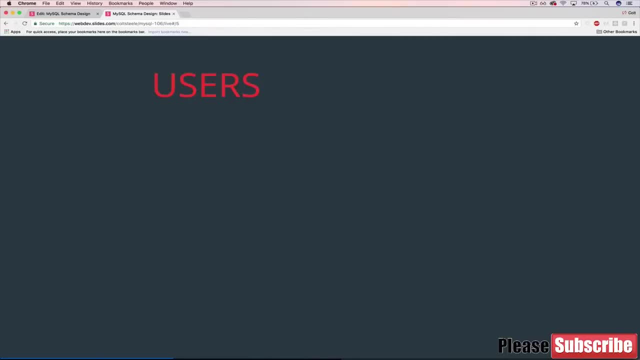 There's a bunch more, But we are going to store information And I'm not saying these are the tables we need. We may need more tables, We may be able to get away with fewer tables, But these are the entities- information we need to store. 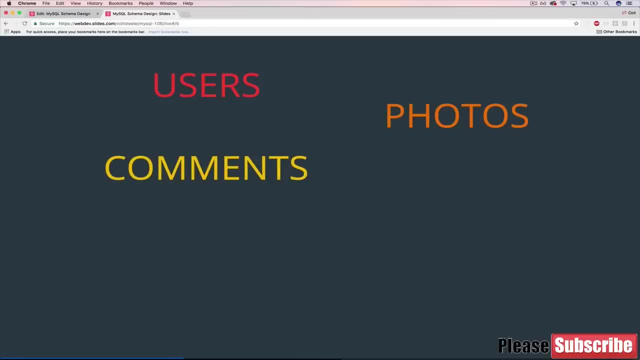 So users, photos, comments on photos, likes for photos as well, Hashtags, which will apply to photos. We're not going to worry about hashtags inside of comments, which you can do on the real Instagram. We're not going to do that. 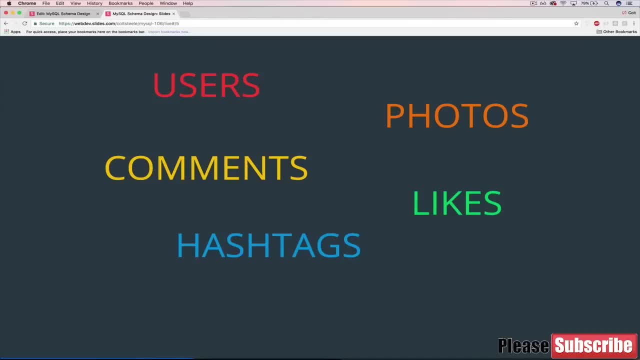 We can talk about how, But it just makes it a lot messier. And then also followers slash, follow ease. It's kind of difficult to talk about the different roles there, but just relationships or friendships or whatever you want to call it. I just call it followers and follow ease, or followings. 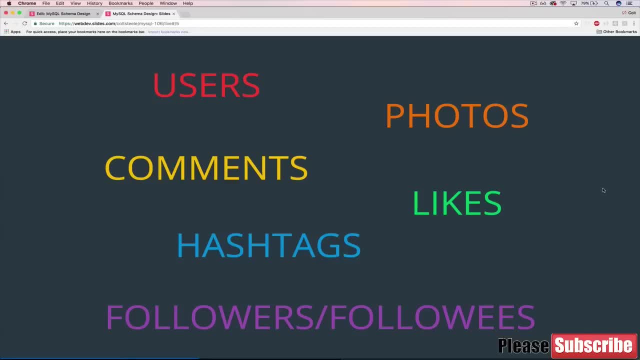 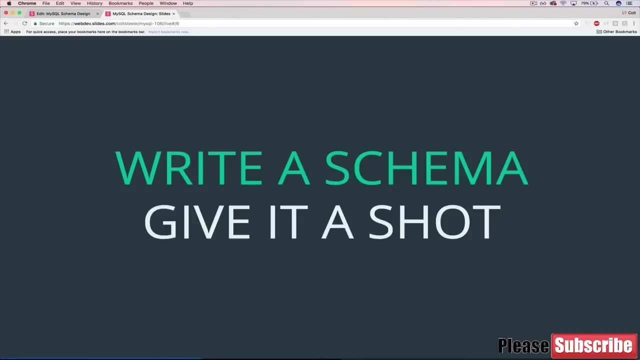 So these are the main things we need to store, And the way that I'd like to structure this is: I would like you to try and give this a shot, so you don't have to actually insert data and do a bunch of exercises on your own. 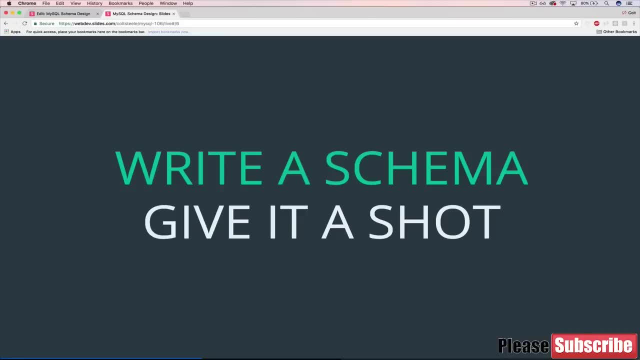 But I'd like for you to At least brainstorm how you would do this. What are the tables you need? I'm going to in the next, in the ensuing six or seven videos, go through each table we need and talk about my solution. 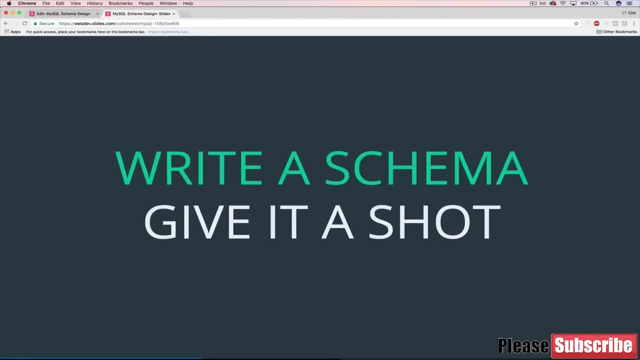 But it would be great if you would take the time to just kind of think about it, jot it down, either draw diagrams out, create a schema file and just write the create table statements, whatever you feel most comfortable with. If you want to get a whiteboard, or post-it notes, whatever works. 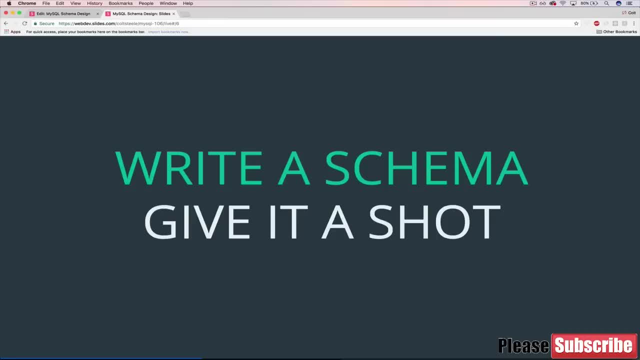 But think about how you would do this if you were creating. It doesn't matter if you're a developer, if you know how to code and other languages or not, But if you were creating an application like Instagram with the functionality we described, what would you sit down and start with for your database and how would you brainstorm? 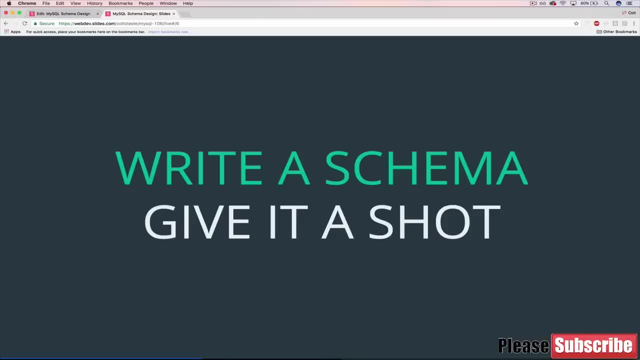 So that's really what I'd like you to do, And then in the next couple of videos, I'll step through in bite sized chunks. I want to make sure that these are short videos, which I know I have said before and maybe have not held up my end of the bargain. 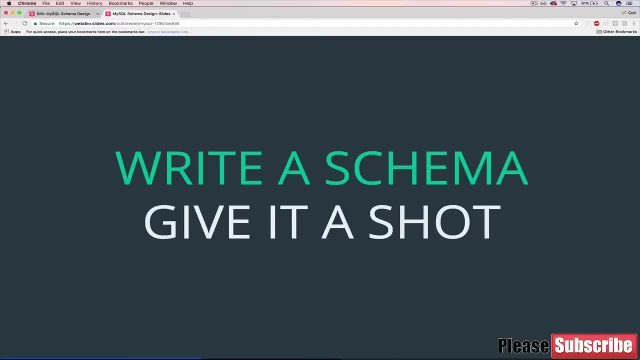 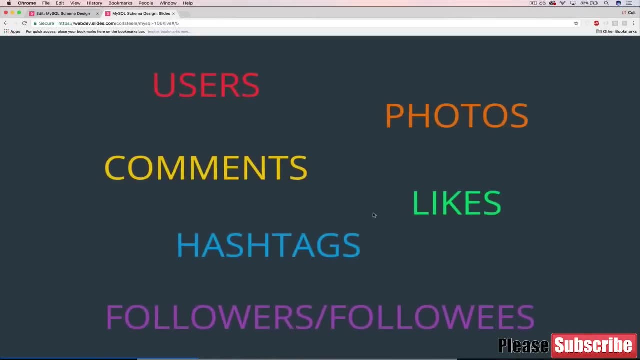 all the time, but these will be shorter And they'll go through my thought process and how I created it. Oh, and before I forget, if you are going to attempt this when you're creating the tables that you need to store this type of information. 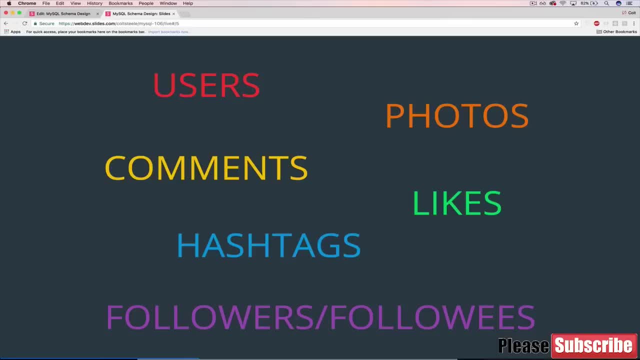 just focus on the core essentials. So for something like users, you don't have to have a username and an email and a password, and I don't know what else Instagram asked for, like a birthday maybe in a profile and all of that. 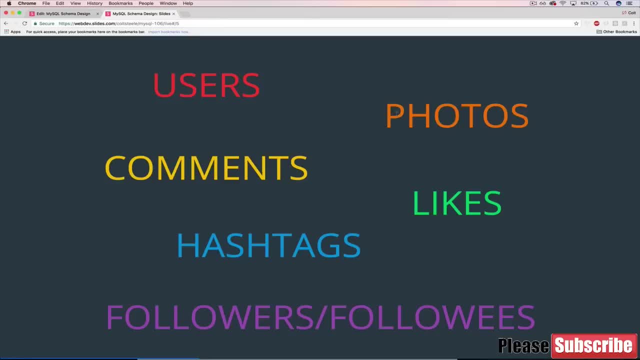 You don't need that, Just the basics, maybe like username and whatever else you need to have it work or have it relate or associate with all the other entities. It's it's easy to add the individual things to a table, like for users. 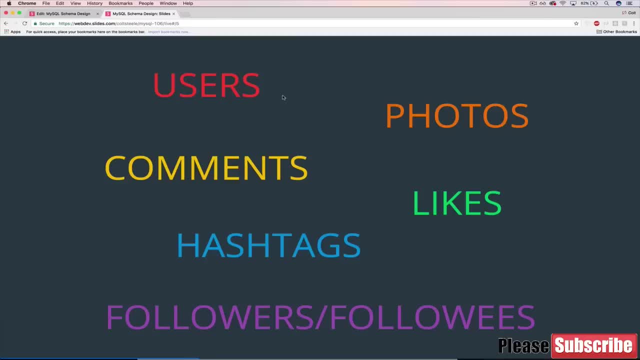 Adding an email column is not hard, but then figuring out how you have users connected to likes, for instance, that's what I'd like you to focus on. OK, so again, you don't need all the information. you can possibly think of, just the key parts. 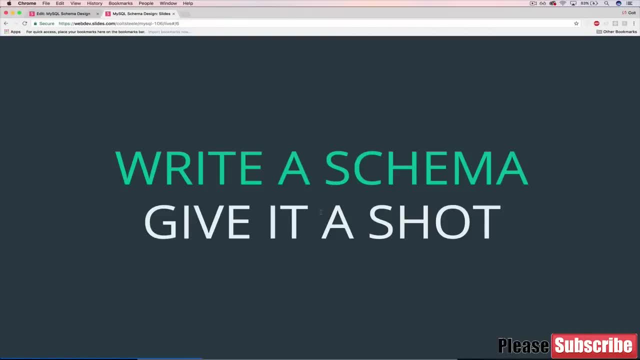 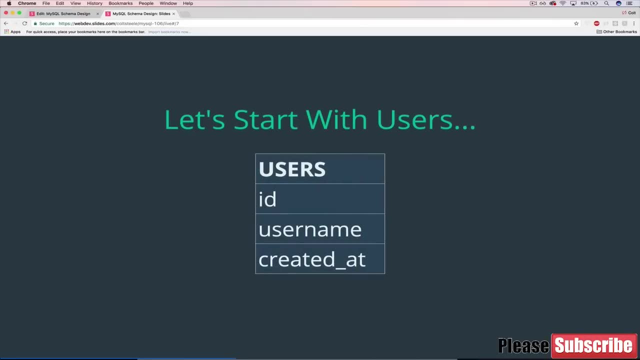 All right. So this is the first video of basically talking about the tables we need and implementing the tables We need for our Instagram clone, And the first thing we'll start with is users. Users is a pretty obvious place to start. I guess another one might be photos, but users is at the core of everything. 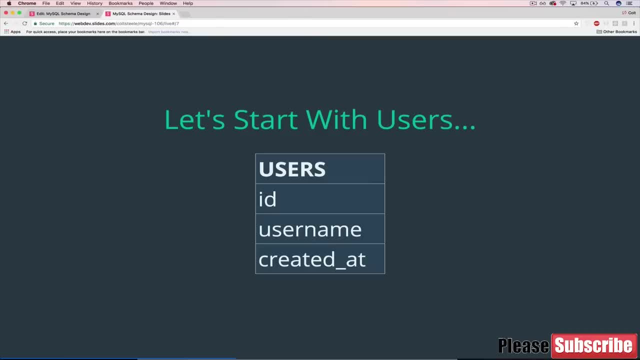 If you think about it, because users are connected to you know, photos are connected to comments, that are connected to likes. They're not connected to hashtags, but pretty much everything else relates to users. So what I'm going to do here is something super simple. 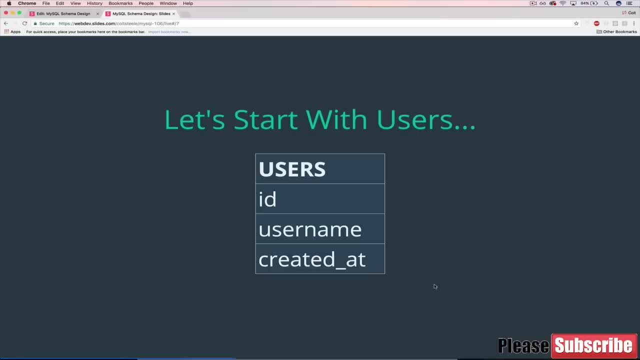 Like I said in the last video, there's a lot more we can store here: email, password, like 20 different things, location, city, IP address, all that stuff. We're just going to focus on the basics. So an ID, a username and a created at and created. that will just be, you know. 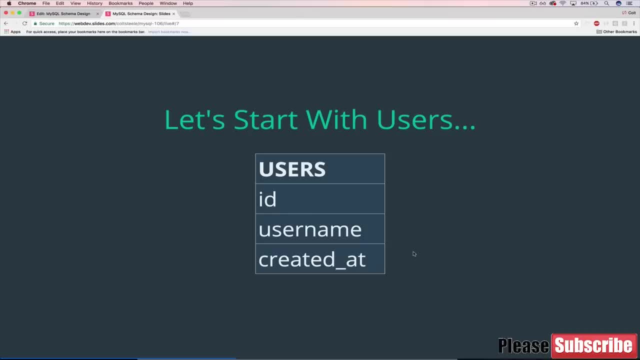 the day, the user or the timestamp when the user signs up, it will have a default value of now or current timestamp. username is just going to be a varchar, varchar and ID will be a primary key And we'll be referencing this ID in other places. 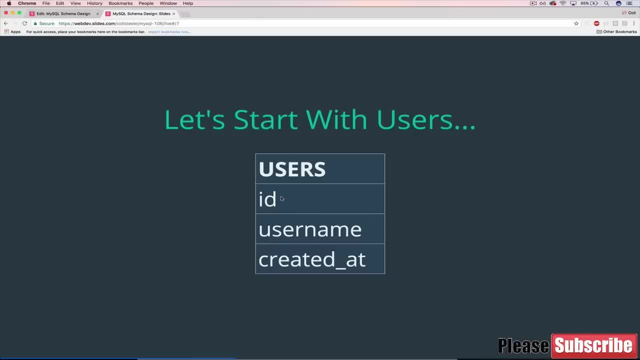 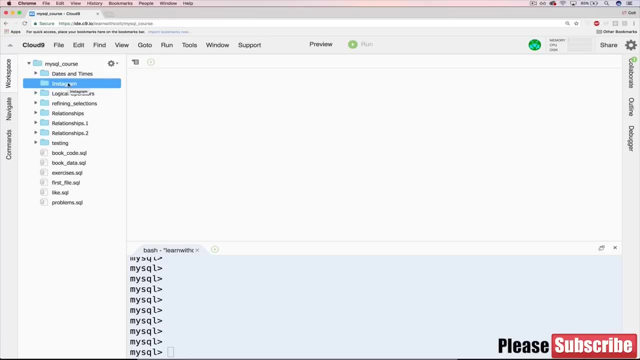 For example, when we talk about photos, photos will have a foreign key referencing the user ID. So we'll go ahead And the first thing I have is just an empty directory. I made just to store this And I'm just going to make a new file. 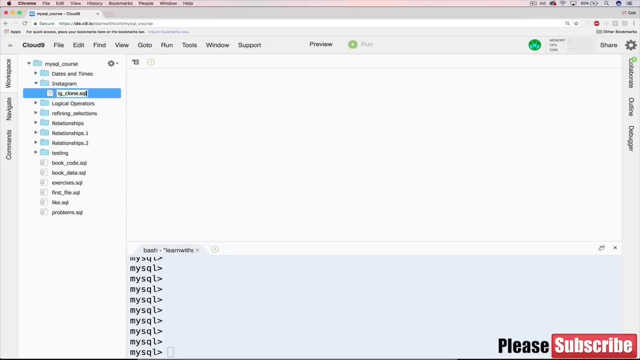 and I'll just call it Instagram: underscore, clone, underscore, clone, dot SQL. I'll open that up And this is where I'll work. So this is where I'll do a create table, users And, like we said, we're going to have an ID. 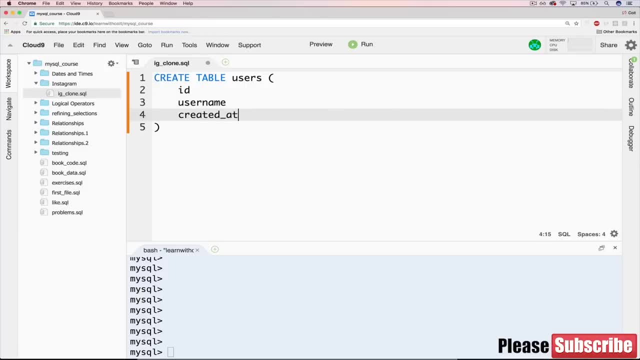 We'll have a username and a created at. So ID is going to be integer or just int. I'll do integer just because I've been doing int, But it's an alias for integer. Good to see both. And we'll have an auto increment and it's a primary key. 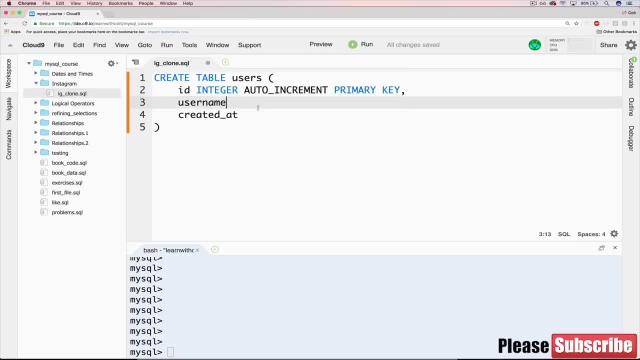 Great Comma. Come back. to Come back to your name, in just a second Created that I'll do timestamp with a default of now And you could also do current timestamp And remember you could do date time as well. Timestamp is just smaller. 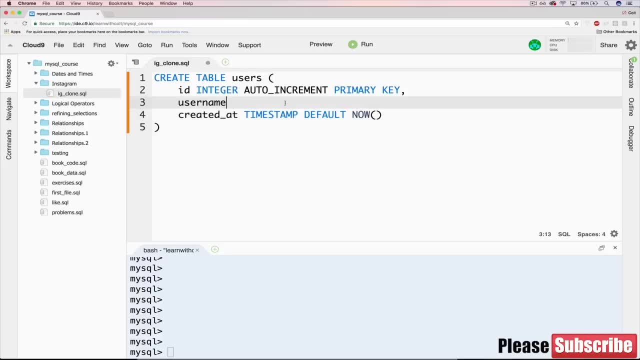 It's easier to store. OK, so then we've got username. We know it's just going to be a varchar 255.. There's another constraint that we could add, though, which is we want username to be unique. We don't want anyone to be able to sign up. 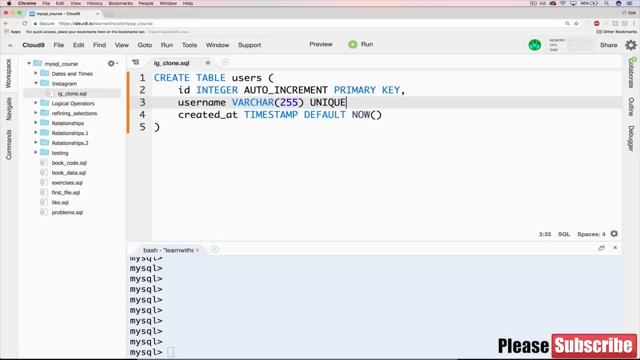 with another with the same username, essentially So we can add unique. And you might be wondering: well then, why would we have ID be the primary key? Why not make username primary key? You absolutely could do that, But if you're going to have a foreign key somewhere referencing username and you're 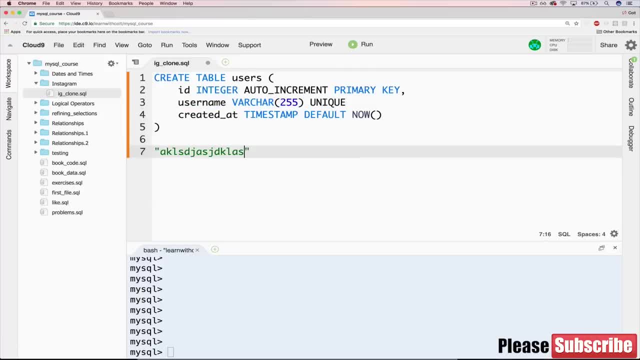 working with a long string. if someone's username is something massive like that, Because we could do 255 characters, that's going to be slower and more annoying to search. potentially- well, not potentially- definitely slower if you have thousands and thousands of entries compared to a smaller integer. 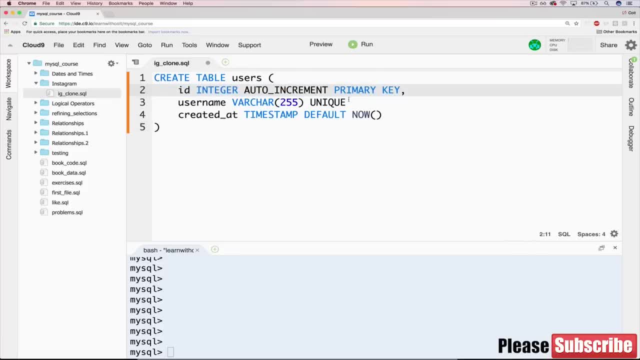 So it's good to have a primary key be an integer. We can still have this unique constraint and we can also add not null. We don't want anyone to be able to sign up without a username. OK, I'm going to go ahead and make a new. 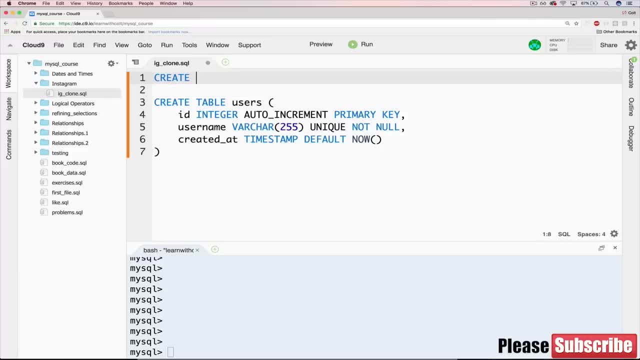 database to put this in, but I'm going to do it in this file. So I'll do a create database and I'll also just call it Instagram or IG clone And then I'll use IG clone just like that. So now, every time I run this file, it's going to make this database. 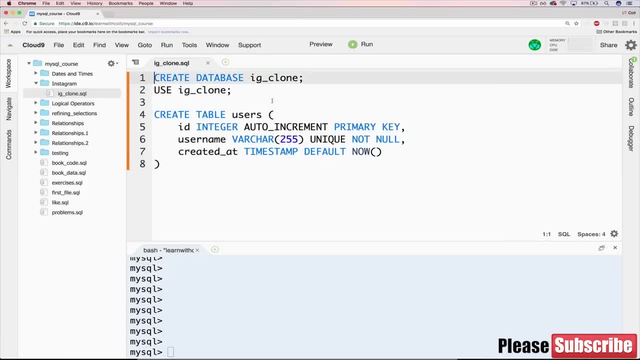 use Instagram, clone the new database and create the table. And the reason I'm doing that is just one: to show you that you can. We haven't really seen using these commands in a file, but also as we go, we may want to rerun this and recreate the users table or another table. 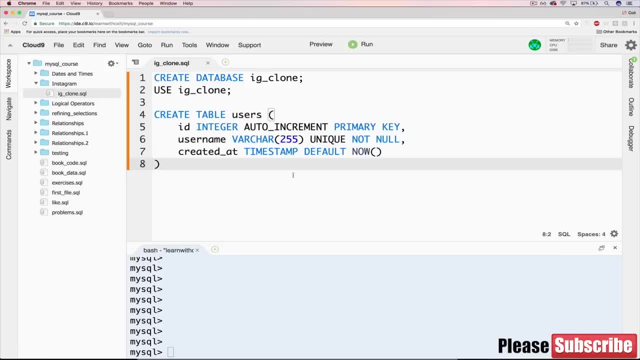 If we realize we messed something up, we need to change something. We're not going to have any data in there yet, so it's super easy just to create the database again, drop it, then create it and then use it and then create the table users. 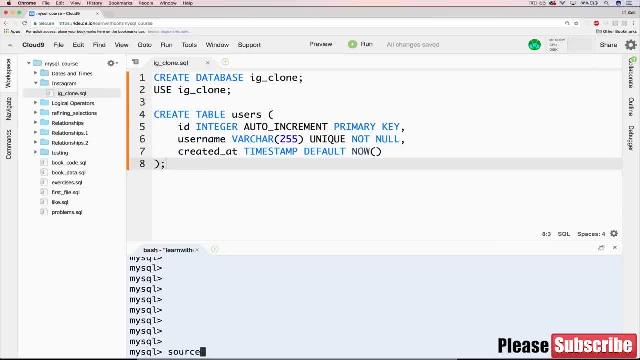 OK. so with that said, let's try this. I'm going to do source And I need to reference this directory: slash Instagram clone dot SQL. OK, and just to double check. describe users. that looks good. OK. so if you are good with that, 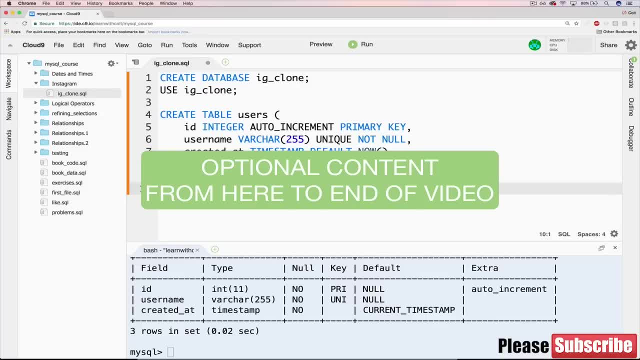 go ahead and move on. next up, we're going to talk about photos, But I will spend a minute or two just adding one or two users so that we can work with them in this section. Remember, in the next section we're going to have a massive data set that I'm going to give you. 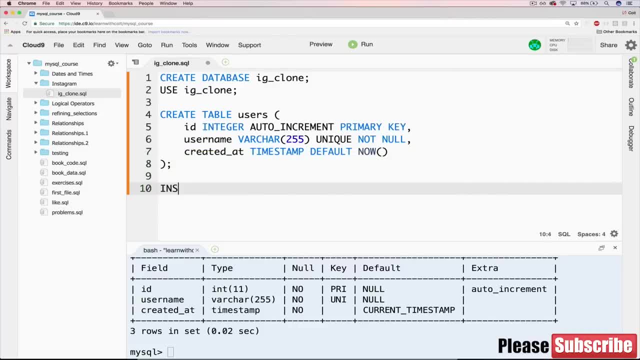 But if we want, we can just play around with some data. So I'll do an insert into users And we'll just insert username And let's just do two or three, so we'll have blue The cat And we could also have- I don't know- Charlie Brown. 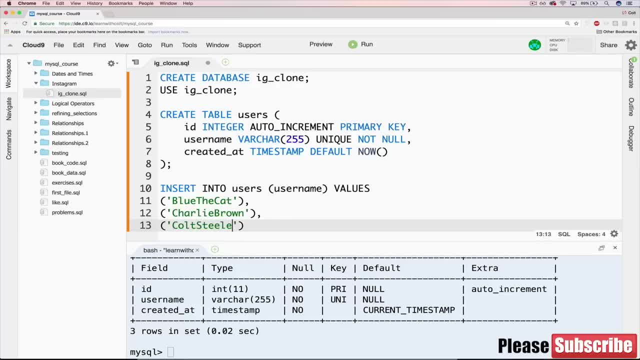 And then I'll just put myself in there just like that. OK, so what we could do now: if I just do, if I resource this whole thing, I'll get an error because it tells me I can't create this database, Instagram clone- It already exists. 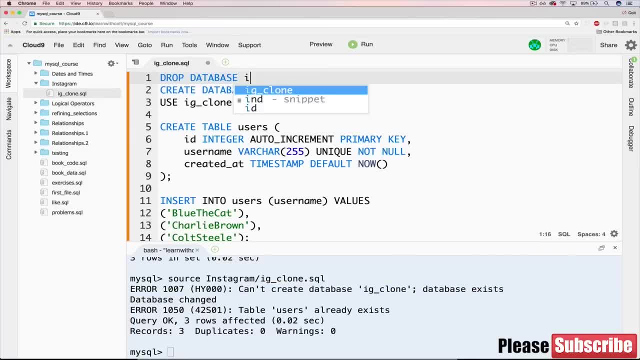 So I could either drop the database first, and I'm going to do that For now. you typically don't want to do that. You don't want to drop a database ever if you can avoid it, But if there's no data in there yet, or if 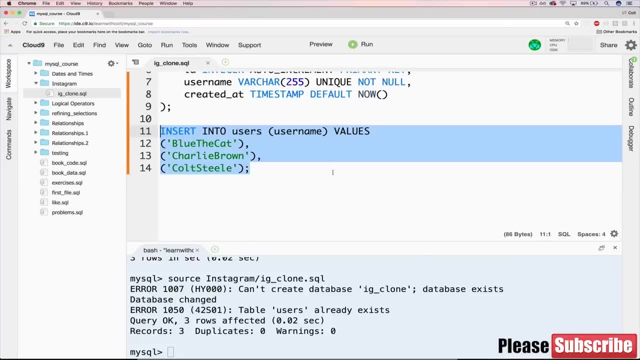 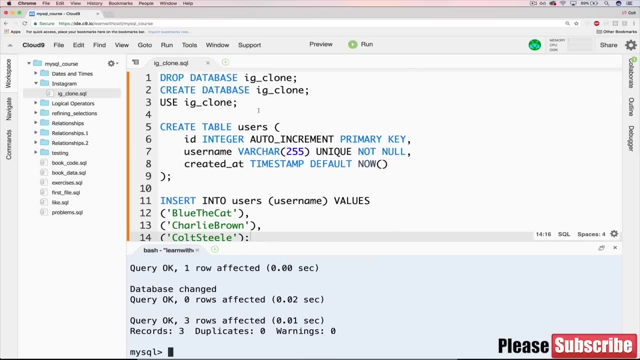 the only data that will be in there is in the same file, like we're doing here, just testing it out. this makes it easy because I can just run this one command. It will erase the database, recreate it and get all the new tables. 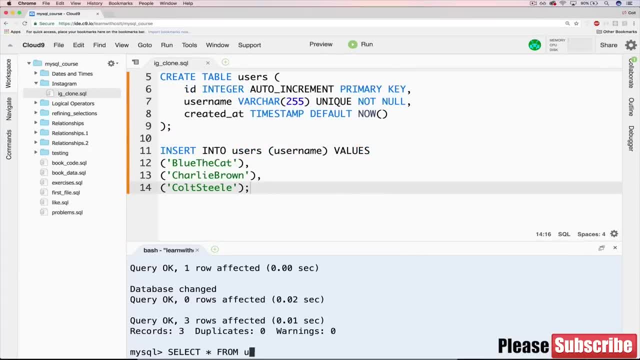 that I need in there as well as the new data. So now I can do a select star from users And there we go. We've got created that in there automatically. The ID is automatic and our three usernames OK. next up photos. 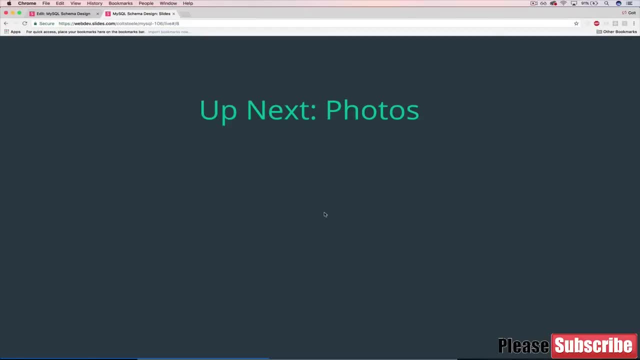 All right, Moving right along here. We're working with photos this time, And the easiest way to store photos is just a single table photos, But of course they need to be related to a particular user who created the photos, So we'll have an ID and all we'll store about an image itself is 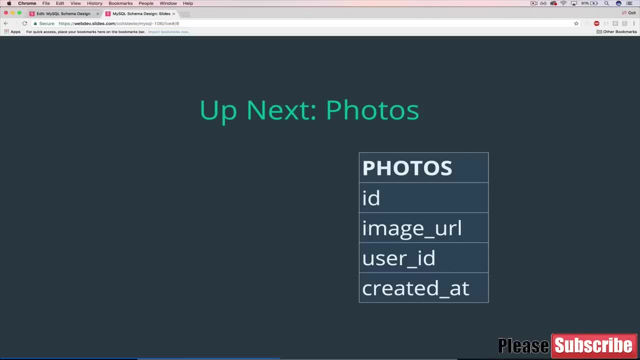 the image URL, which will just be a string. We could have added a caption as a varchar- excuse me, not a string. We could have added a caption. We could have added location data on Instagram. You can say where it was taken. 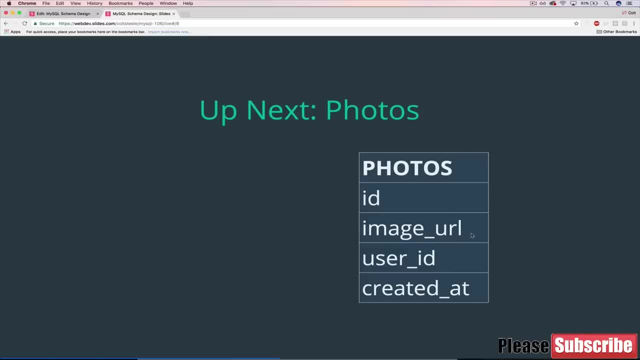 You know, there's all sorts of things that we could do, But we're just focusing on image URL in our case. And then the user ID- very important foreign key pointing to usersid- And then we also have created that, just like we had with users. 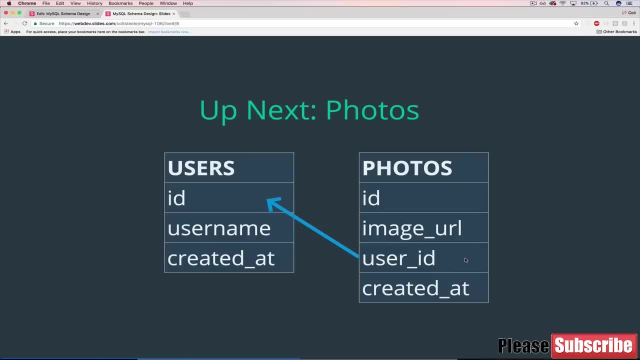 Just a nice way to be able to sort photos by most recent to least recent or figure out the first photo somebody posted, Or if one photo is posted before another, if one looks like it's. this is actually happened to me. People take a photo of mine and repost it, claiming that it's their own. 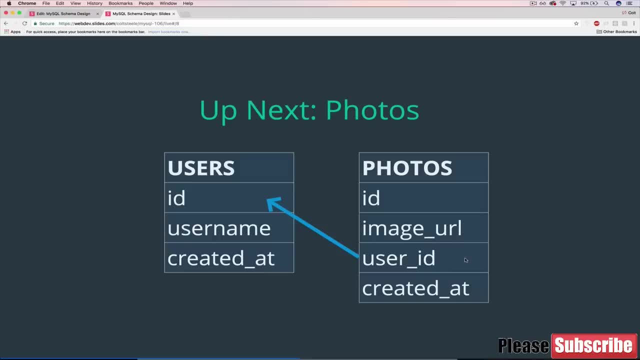 It doesn't happen often, but two times, actually by the same person, And the person actually flipped the image like mirrored it posted. it claimed that it was their own, but of course I could just show that mine was posted first. 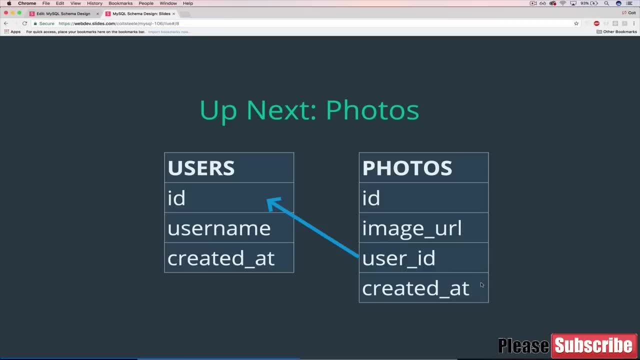 Thankfully, Because there's a date. I mean, it didn't really matter anyways. Right, It's just photos on a social network, But still having that created, that in there helped me there, So let's implement it now. It's pretty straightforward. 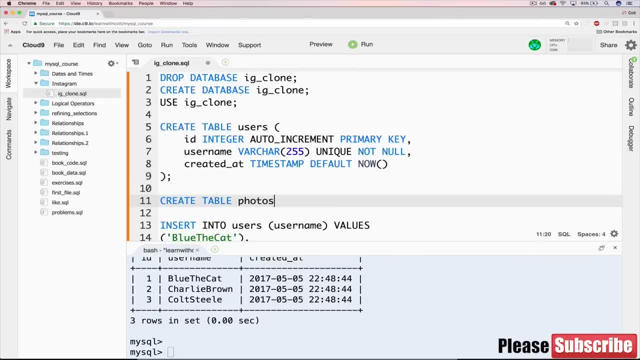 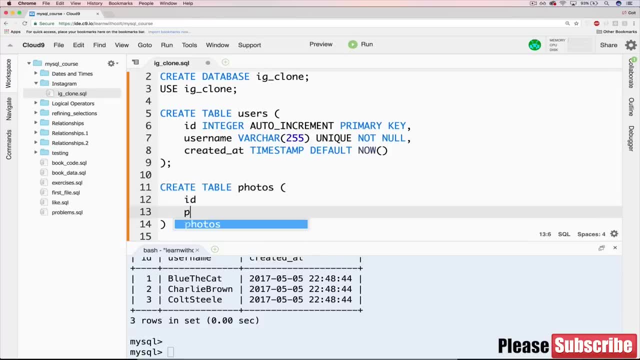 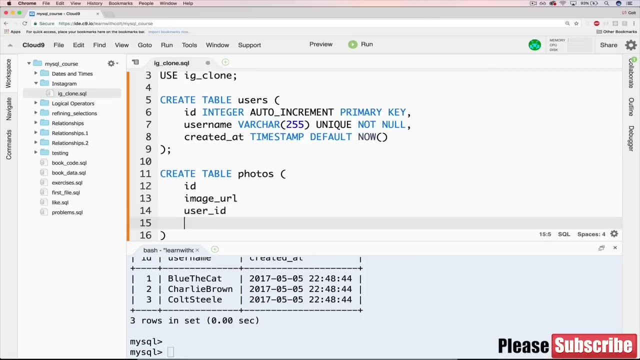 Just create table photos. We're going to have an ID. We'll also have our photo or image URL, whatever we want to call. that will have a user ID and then created that. So ID is an integer or an auto increment. Primary key. 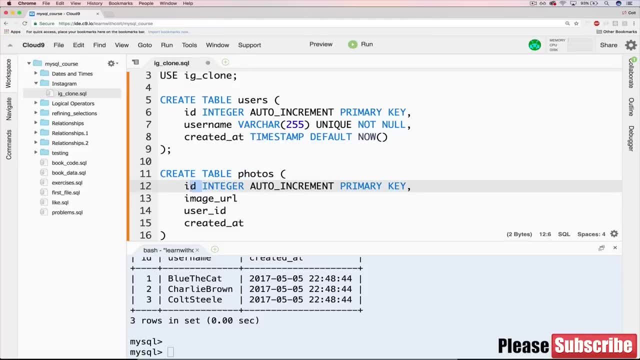 will be referencing photos that ID from other tables, because things like comments are associated with a particular photo, or likes are, and tags as well. So we need that primary key there. Image URL will just be a varchar 255.. But we should add, not null. 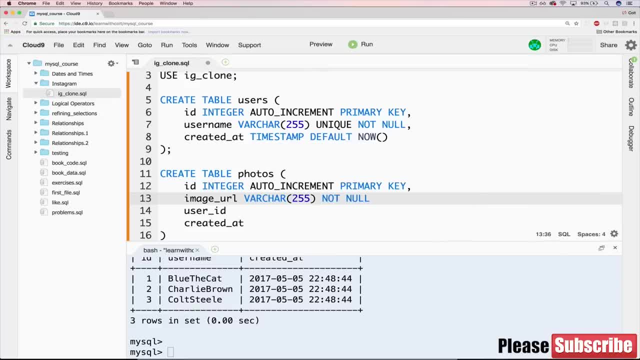 We don't want that to be empty or to be null. That's a big problem because there be no photo to display And then user ID that will be an integer And let's also make that not know. a photo needs to be associated with the user. 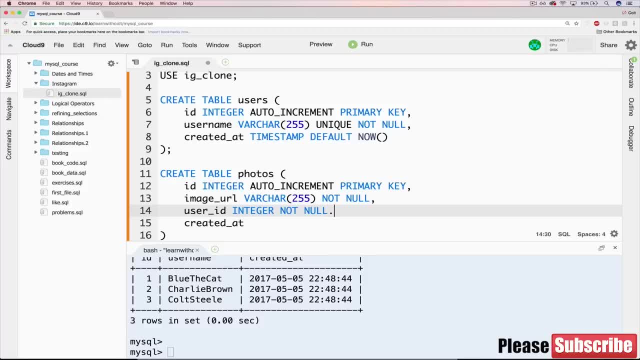 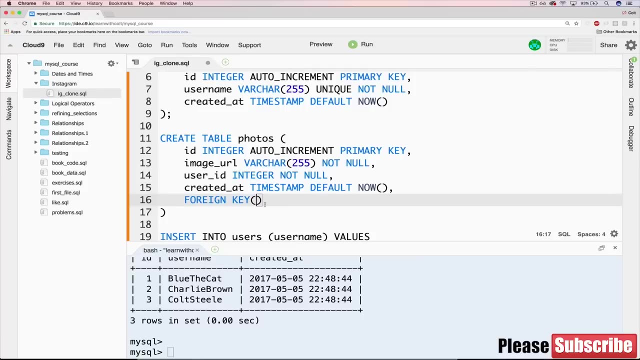 We can't have an orphan photo that has no user and then created. that will just be another timestamp with the default value of Now the time is created, But we still need one more piece, which is our foreign key constraint, which is going to pertain to user underscore ID. 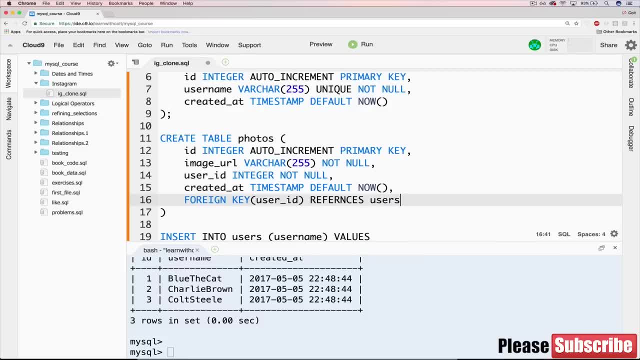 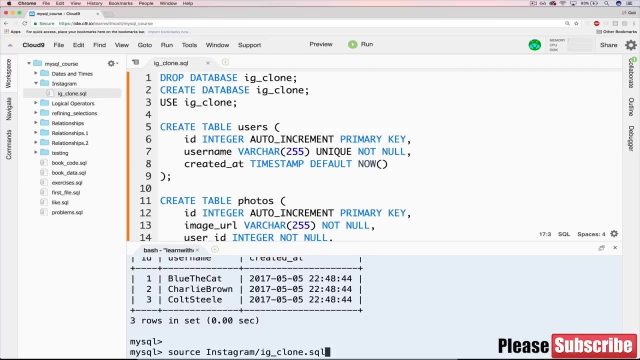 which is referencing or references the user's table, The ID field. I spell that reference. There we go OK And that will create our photos table. So if I just resource this whole thing Now, if I do show tables, We have both tables in there. 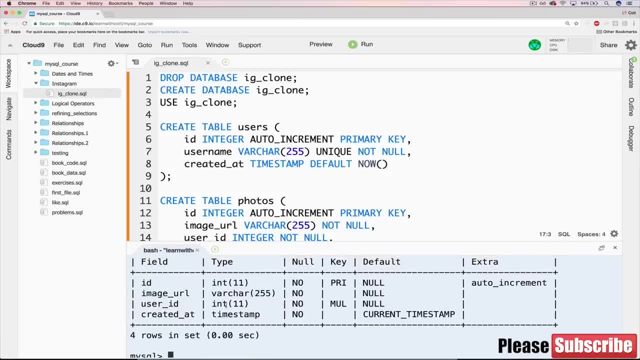 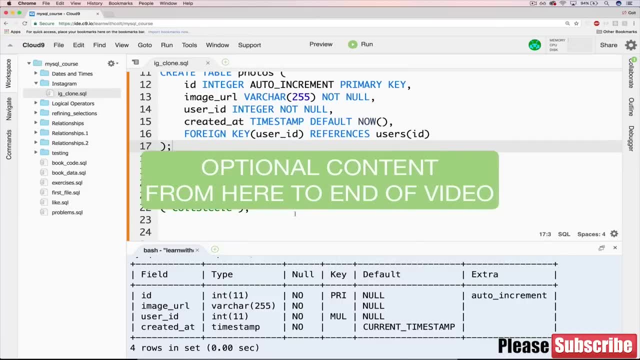 If I do a describe photos. we've got photos there. everything looks good And just like before. if you want to stick around, I'm going to insert one or two photos in here associated with our three users, But I'm done with creating the schema. 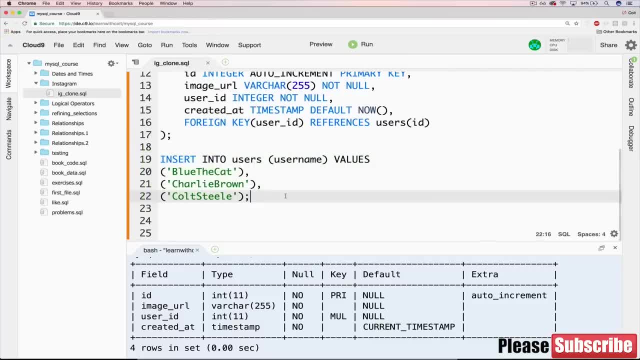 So feel free to move on to the next one, which is comments. But if you want, you can stick around as I do an insert into photos And we'll just do an image URL And a user ID. Those are the two things we have to supply ourselves. 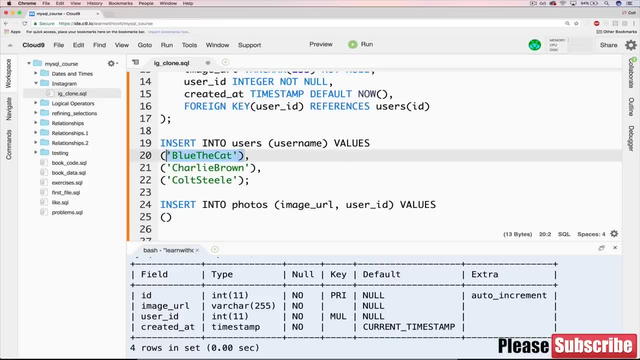 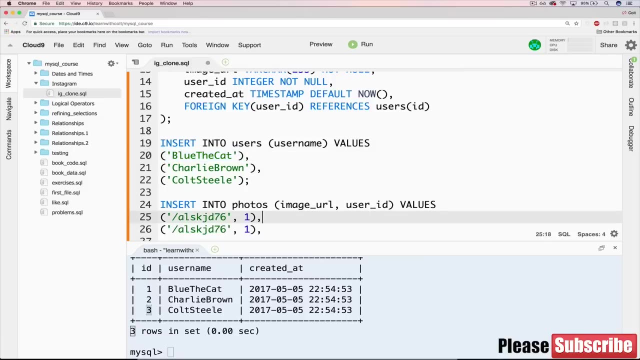 Values and our first one, let's say Blue submits it and we'll come back to the URL, But Blue's ID is going to be one And if we weren't sure, we could do select star from users. You can see: Blue is one, Charlie Brown is two and Colt is three. 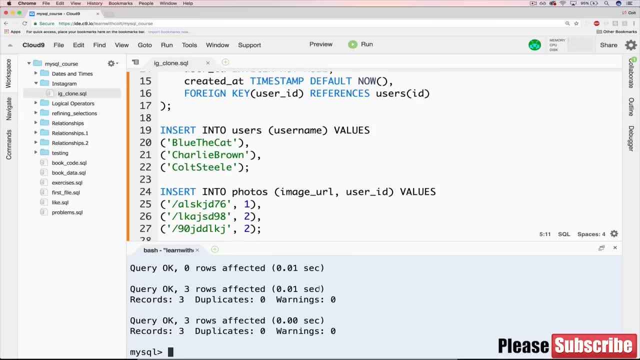 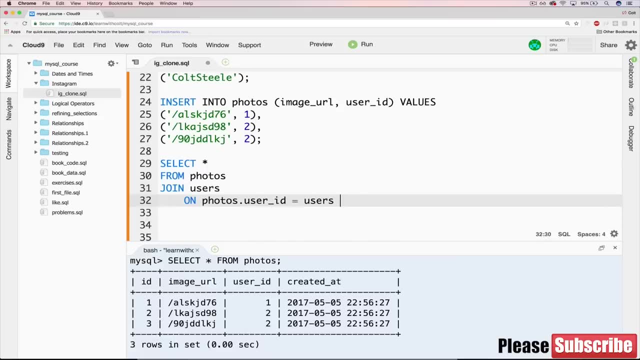 So we'll just do something silly. Let's just say the URL is just random like that. I'll duplicate that a couple of times In Cloud nine it's command shift D or control shift D on a PC. And then here's another random thing. 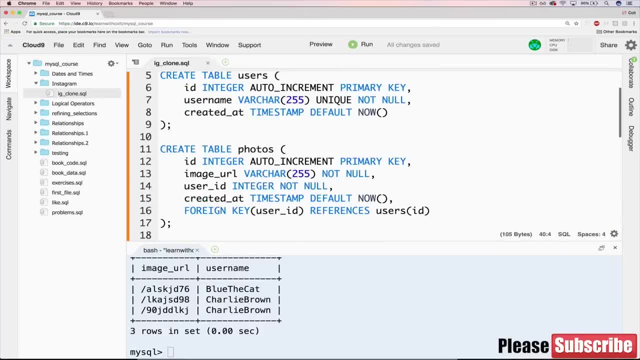 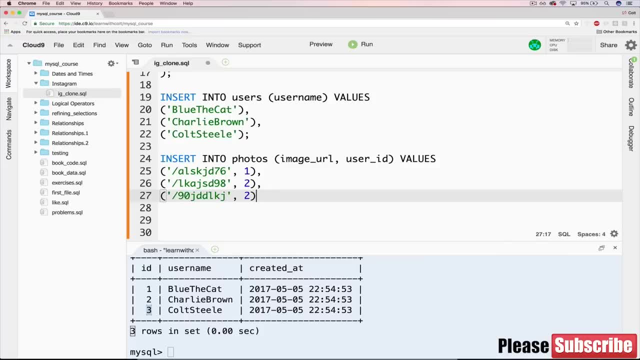 This time it's submitted by Charlie Brown. Let's say Charlie Brown has another one as well, like that. Okay, And I haven't submitted any photos. that should work If we run our source again this time. so it dropped the database, recreated it, switched to it with the use. 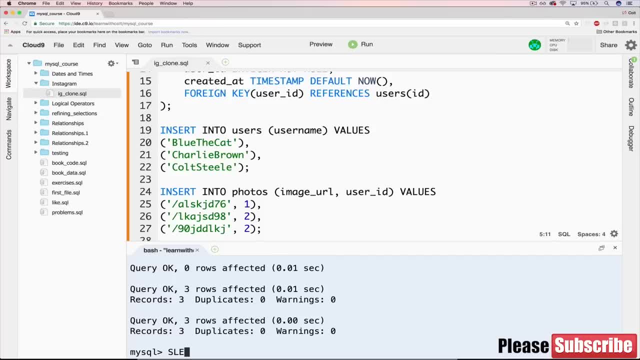 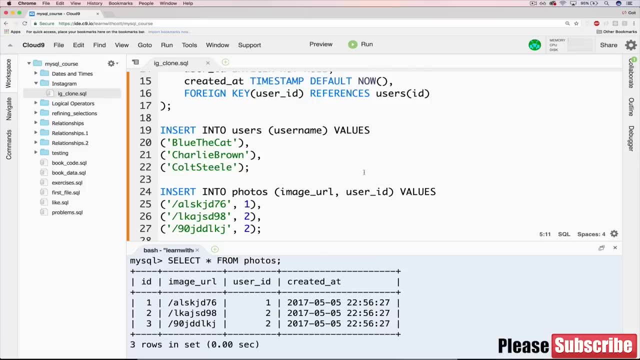 command created our two tables, inserted all of this data. Now, if we can do select star from photos, and we should have three simple photos there with a user ID- We're now at the point where we could do a simple join, if we wanted to, to figure out who posted these photos. 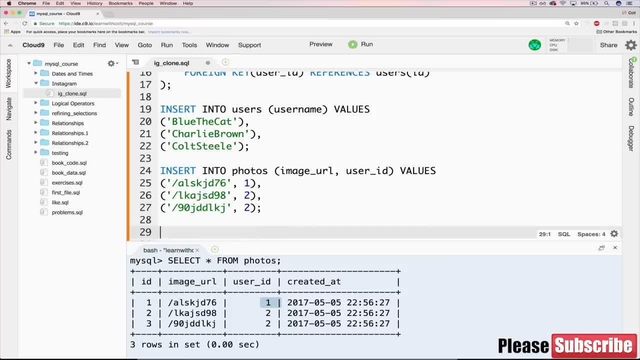 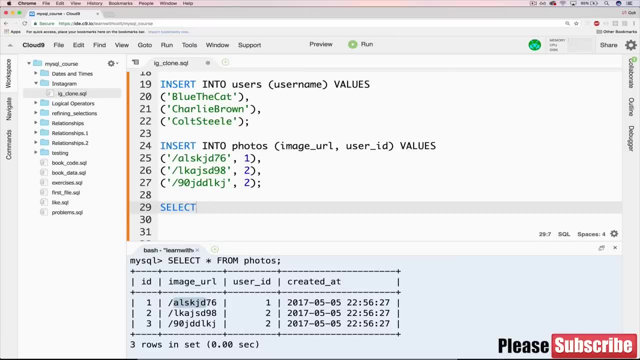 So again, definitely. if you feel good about this, move on and don't waste time watching this. But if you want the practice, we could just do a select. Let's say I wanted to have the image URL created at and the name, the username of the person instead of the user ID. 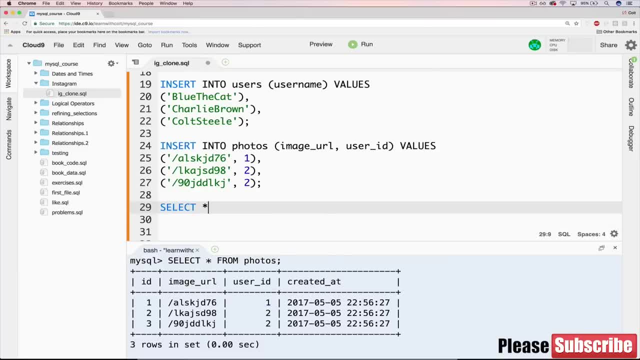 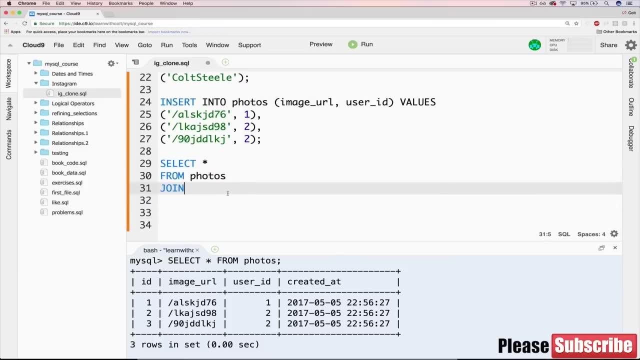 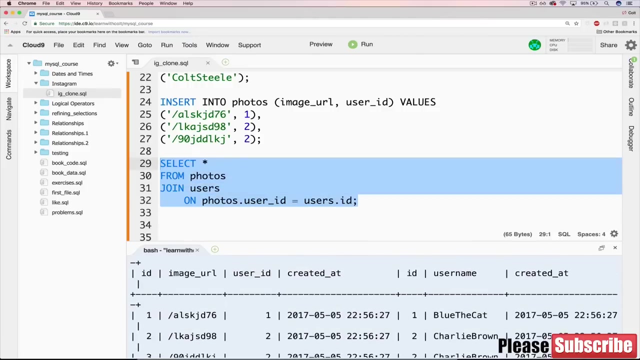 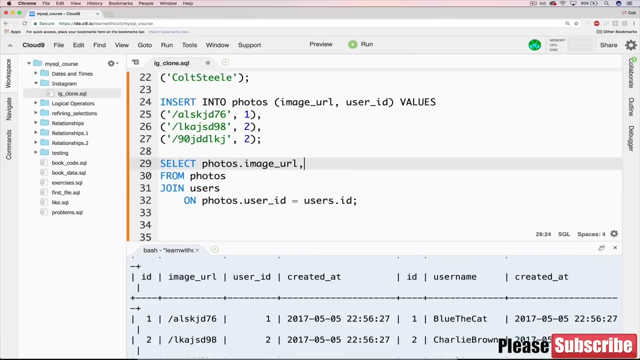 So we'll just do a select star to start from photos join and we'll just do a default inner join users on, and we're going to do it where photos dot user ID equals users dot ID. So if we start with that, There's a lot there so let's send it out to just be photos dot image URL comma. 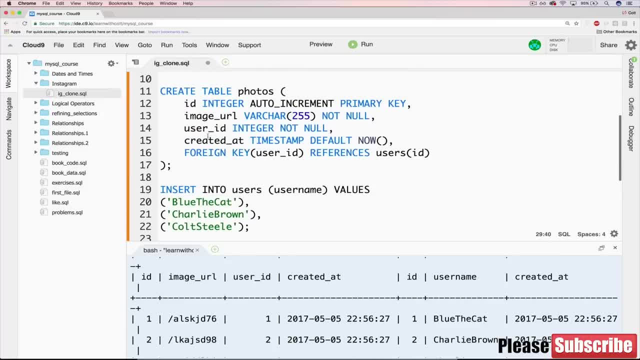 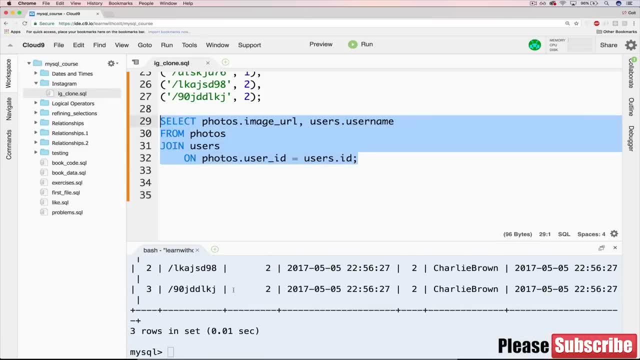 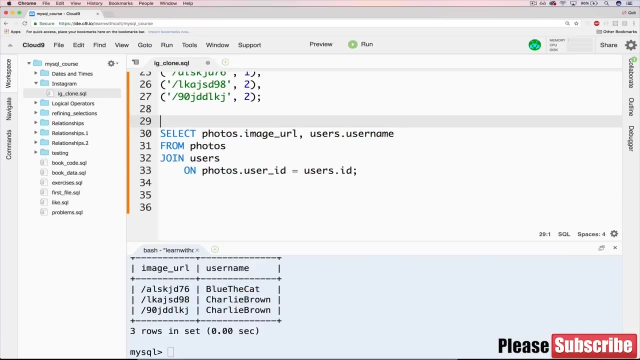 users dot username. that would use username. Yes, just like that. Copy it. OK, now we can see. the cat created that and Charlie Brown created those two. All right, And what I'm going to do, just to set a pattern for the next few videos, is move. 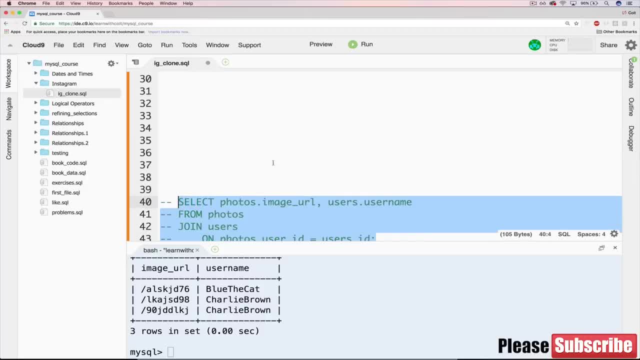 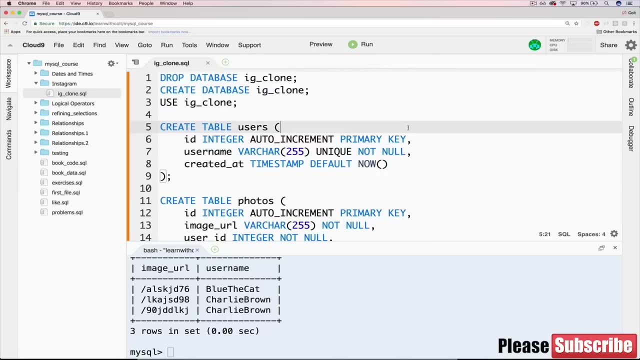 these joins and things that I'm just playing around with down to the bottom and comment them out. We don't want those to run, but I'll leave the insert statements here, as well as to create tables. All right, Moving on. All right, So we're moving on now to comments. 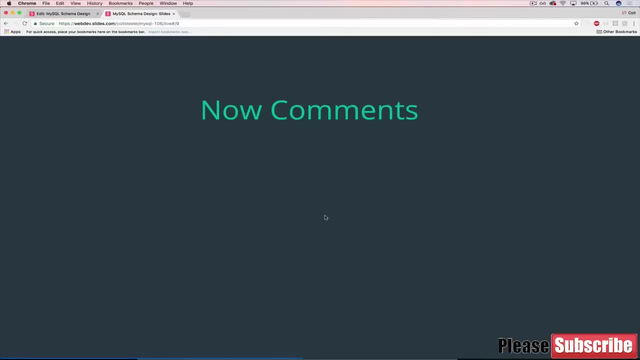 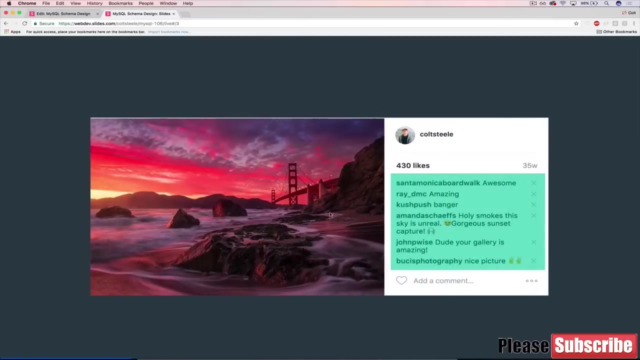 And we did users first, and photos for a reason. One is that they're simpler and essential to Instagram. but also comments is going to rely on them, because if you think about how comments work, if we go way back here, these comments, Over here, this handy green box to draw, 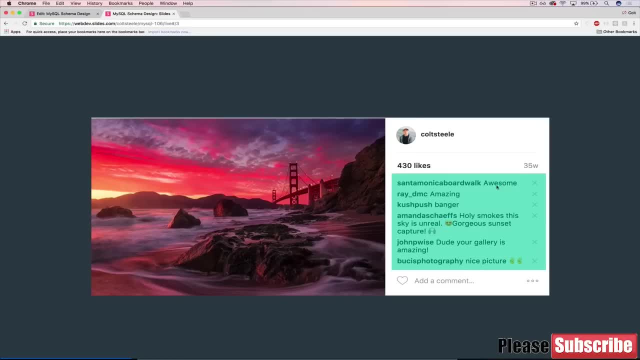 your attention, are written by somebody, right, so it's not just a comment like awesome or banger, but there's also somebody who wrote the comment. So there's some association there. So a comment needs to be related to a user, But then these comments 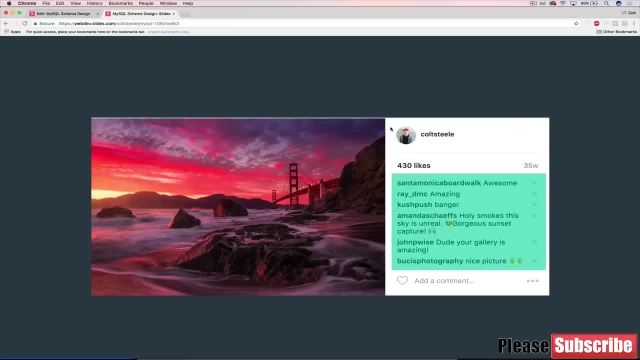 are related to a particular photo. These comments here are for this photo, not this one right? So they're not just floating in thin air, but they're also related to a photo, which means we're actually going to have two foreign keys. 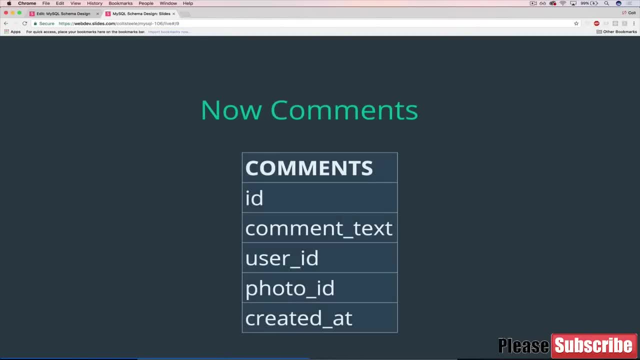 So it looks like this. We have a comments table. comments will have an ID primary key, our comment text, which is just, you know, the text of the comment. I didn't want to call it text because that's a reserved word in my SQL. 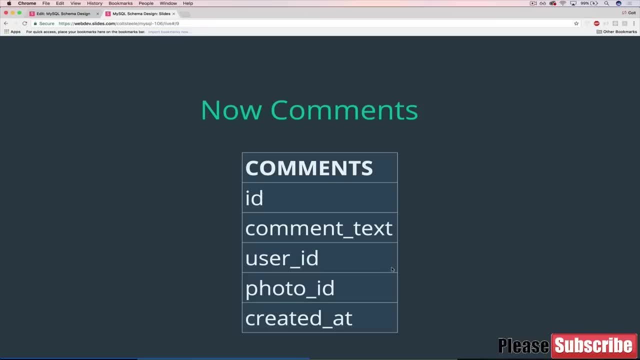 Even though it might work for you, it's just not a good idea to mess with that. And reserved word meaning that text is a particular data type. It's something that's used in my SQL in the language, So naming a column in a table is not a great idea. 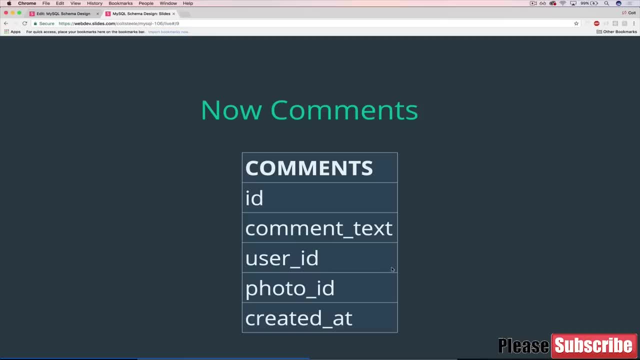 It's like naming a column integer. Okay. then we've got user ID, which is a foreign key related to the users ID, So that's how we know who wrote it. Then we've got photo ID, which is also a foreign key, this time. 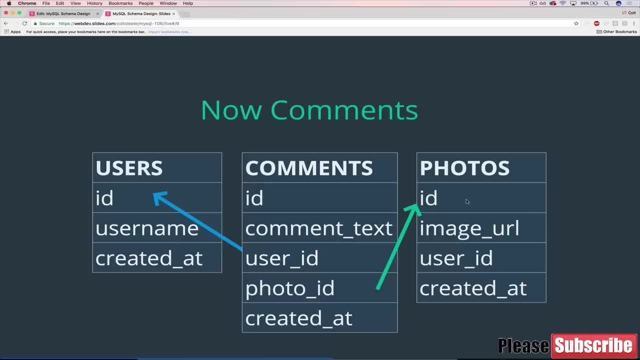 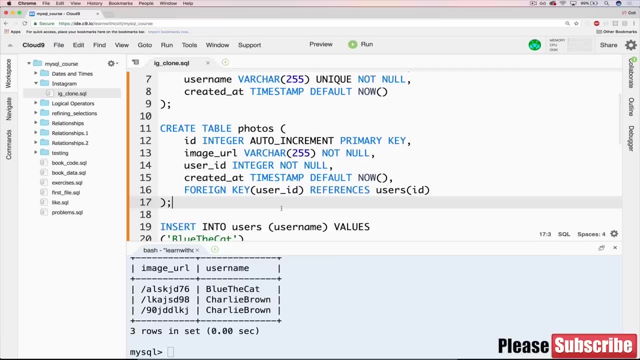 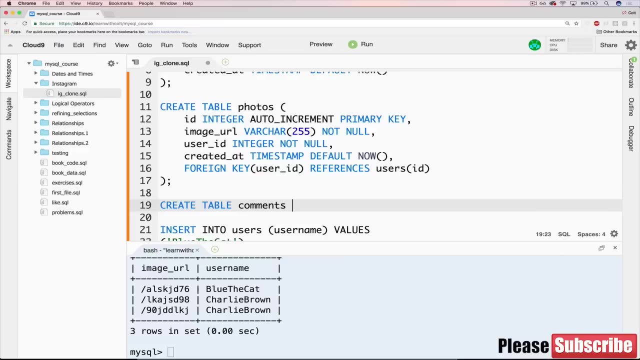 to photos, that ID, which is how we know which photo the comment is on. And then we've got our good old friend created at. So let's hop over to Cloud nine. Do it down here after photos. So we'll do a. create table comments. 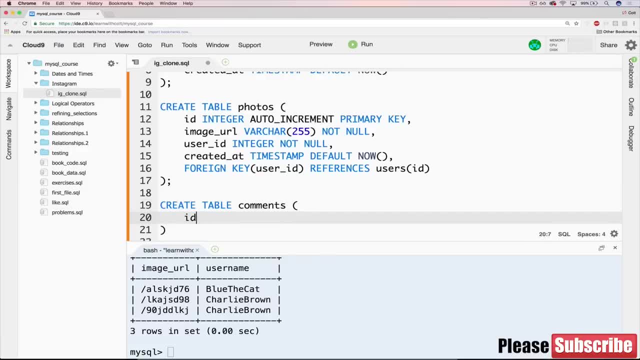 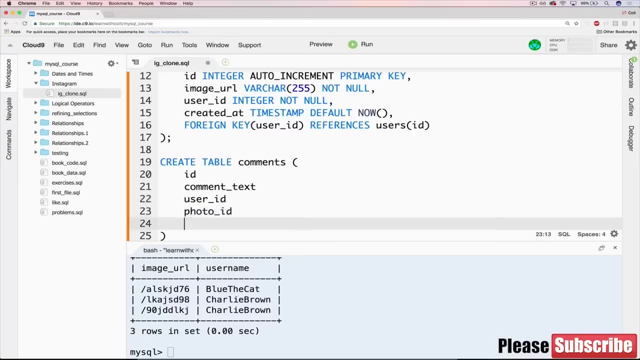 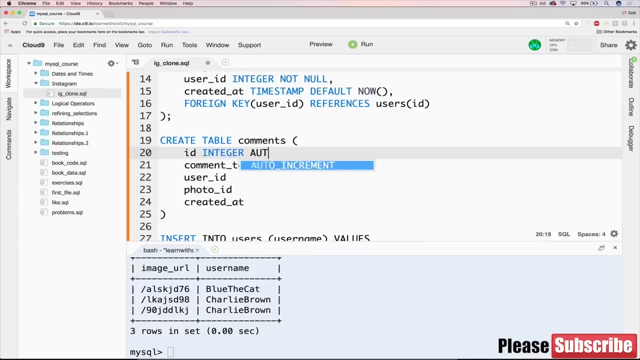 And our main things. we've got ID, we've got comment text, Then we've got user ID, photo ID and created at. So we'll start with ID, We'll do integer auto increment, primary key: Pretty standard comment text will just be. 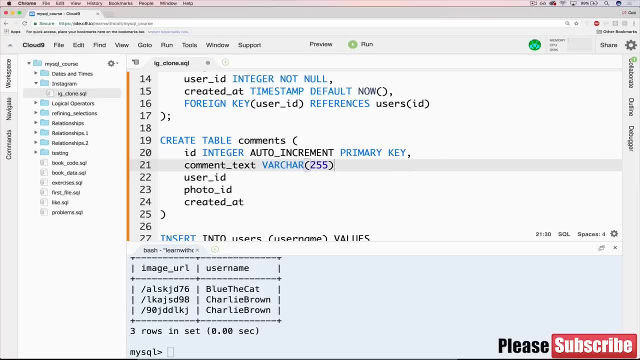 Varchar 255 as well, as we want to make sure it's not null. We don't want anyone leaving empty comments. If you try that on Instagram, it just won't post it. Then we've got a user ID, which is just an integer. 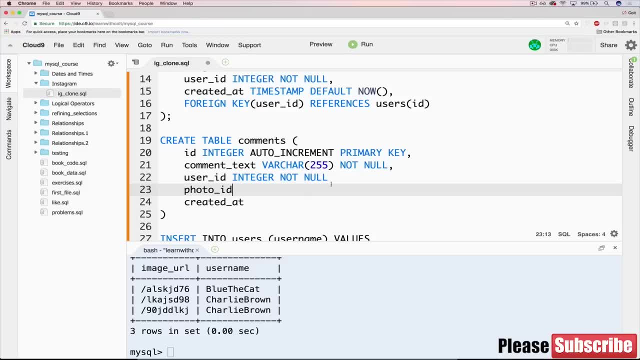 But we also want that to be not null. We don't want to have a comment: that's an orphan, that's not related to a user. Same thing for photo ID: It's going to be an integer. We also don't want it to be not null, or we don't want it to be null. 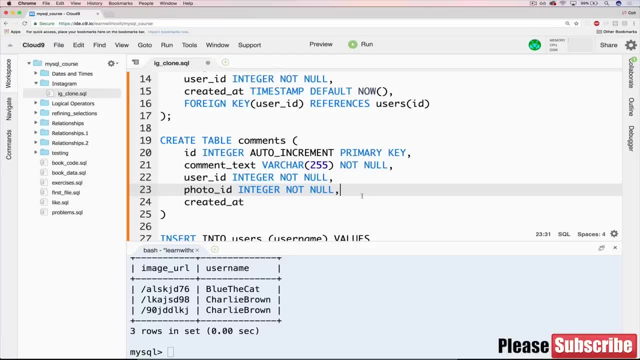 We want to make sure it's not null, because then we'd have another type of an orphan: a comment without a parent photo. So we have these two relationships here: User and photo are related to comments, OK, and we don't want either one to be null and then created at good old timestamp. 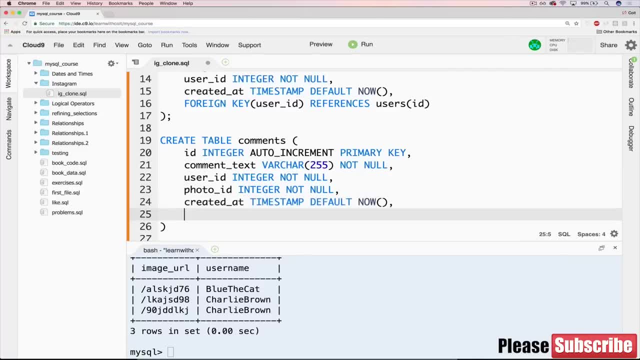 default now, but we're missing our foreign key constraints. So foreign key and we'll start with user underscore: ID references users ID comma. Then we've got another foreign key. This time we're working with photo ID, which references: 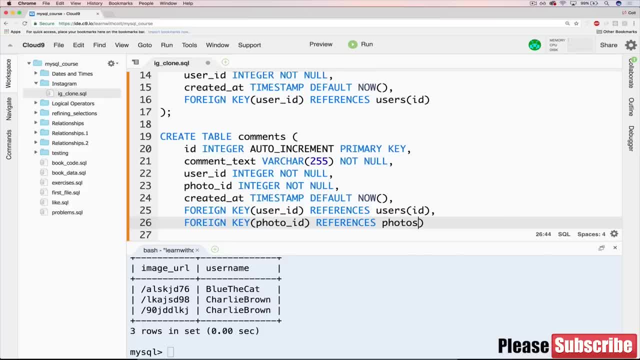 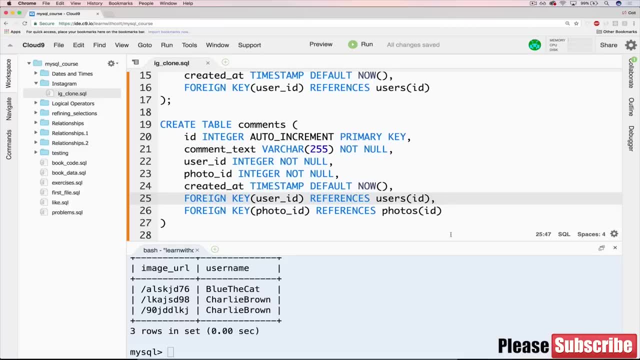 Oops, Photos ID. There we go. OK, so just to make sure I don't have any typos here. I had my semicolon and I'm just going to resource that. if I can find it, Here we go. Looks good so far. 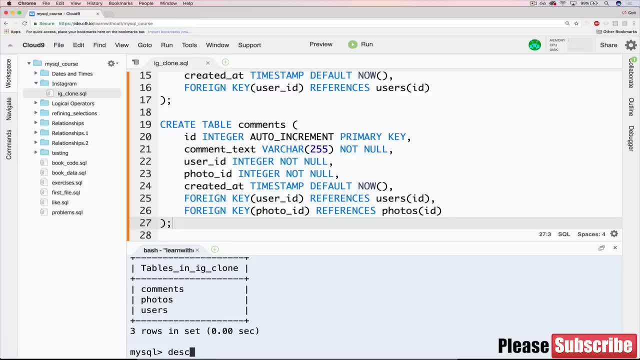 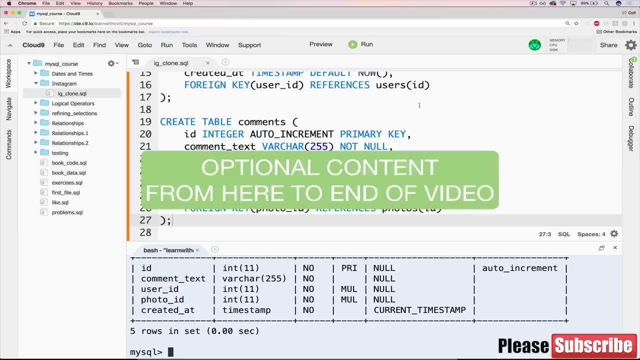 If I do show tables, I've got comments and I can do describe comments and we're good, All right. So, just like the last few videos, stop here If you feel good With this, if you want to see me insert some data and see how we relate things when we actually insert the data. 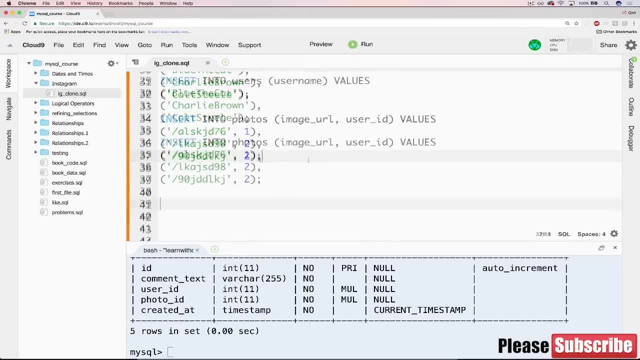 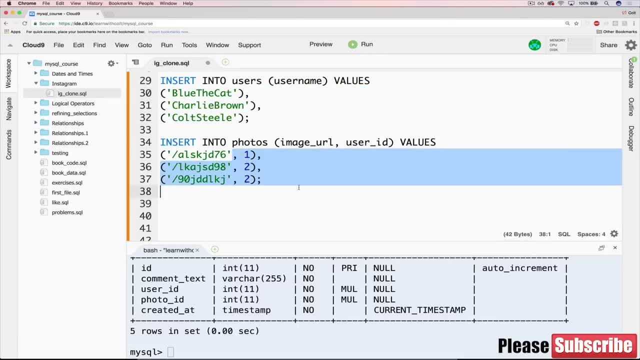 I'm going to do that, But, of course, move on if you feel comfortable. So if you're still here, what I'll do is insert a couple of comments between are related to these three users and these three photos, And this is where it gets kind of difficult to keep everything straight. 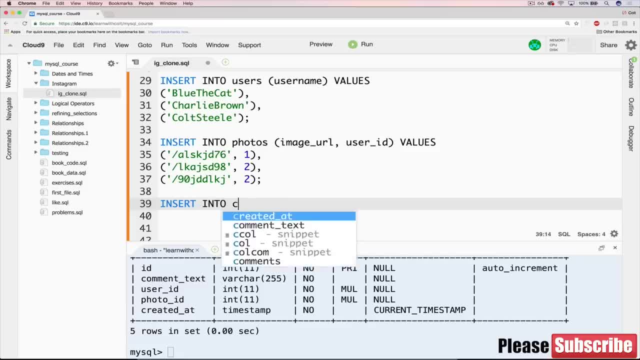 keep all the ideas and everything straight in your head. So we'll do an insert into comments and we'll have comment text. Then we'll start with the User ID, who's posting it, and then the photo ID values. So let's say our first comment is going: 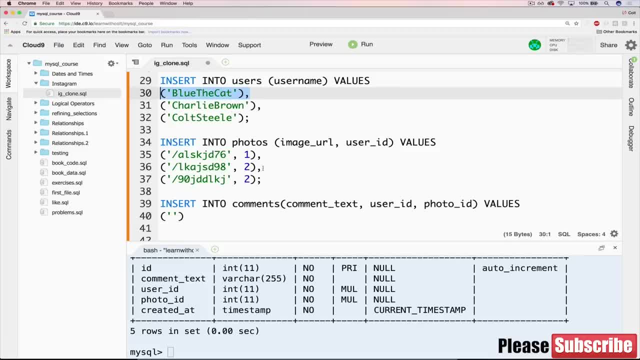 to be blue commenting on This photo here. saying this is her comment is just me out. OK, so that's the comment text and the user ideas. who's saying it? Blue the cat has an idea of one And I just you can tell, because we 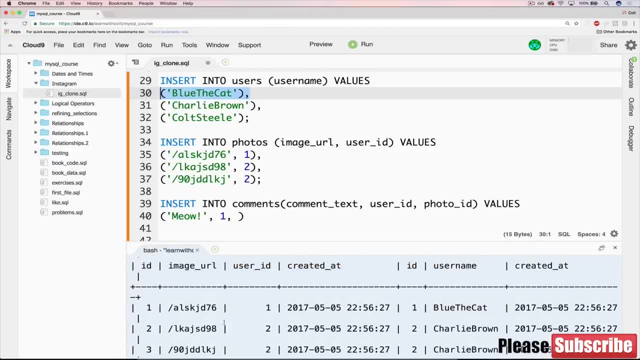 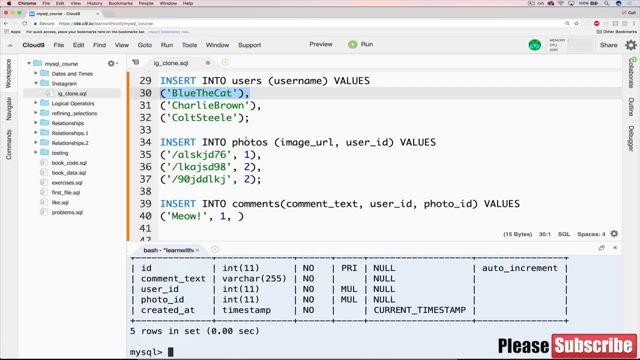 inserted her first. but of course, if we went back to our select way back here, You can see- oh no, you can't see there. you can see here her ideas, one OK, and then the photo ID will just say she's commenting on this one here. 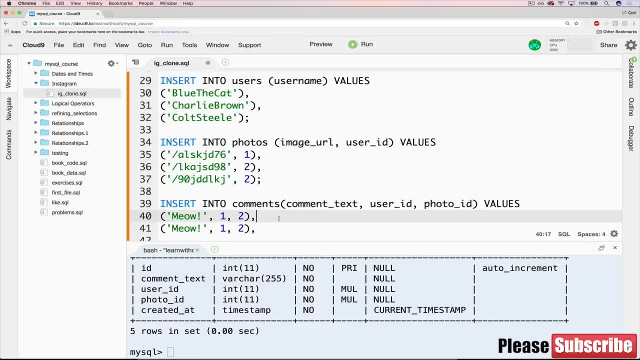 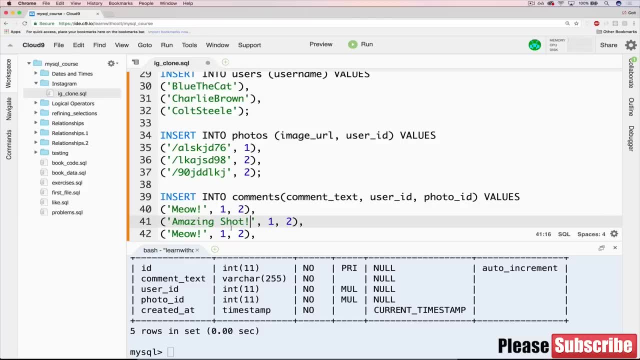 The photo idea of two And I'll duplicate that. So let's say somebody else commented and say someone says amazing shot On the same photo, photo here, And let's say I commented on that. So that would be my user ID three. 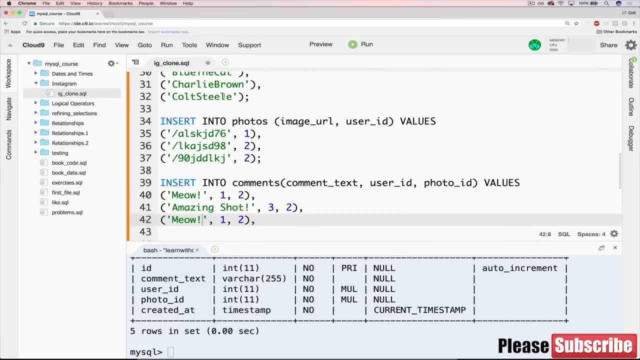 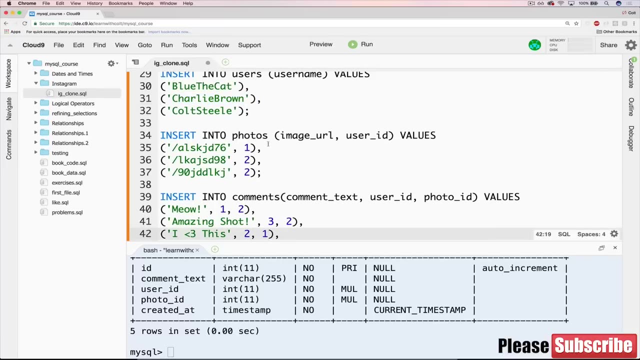 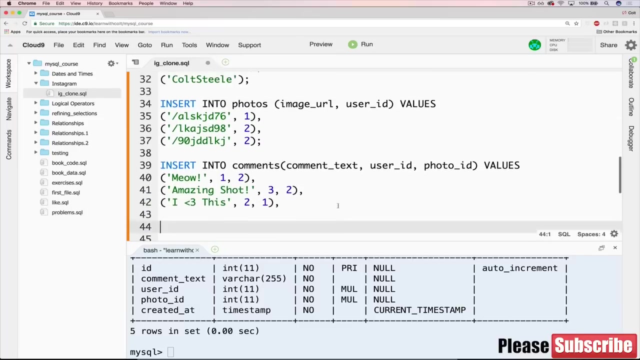 And we'll do one more this time. Let's say Charlie Brown is commenting- I heart this. and Charlie Brown is user ID two. And let's say he's commenting on the first photo that was submitted by blue with user ID one. So you can see how it gets a little bit crazy. 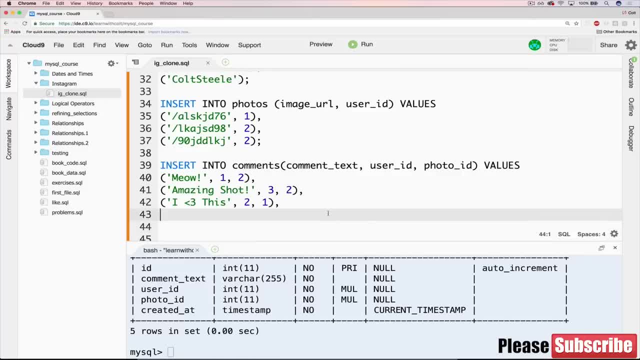 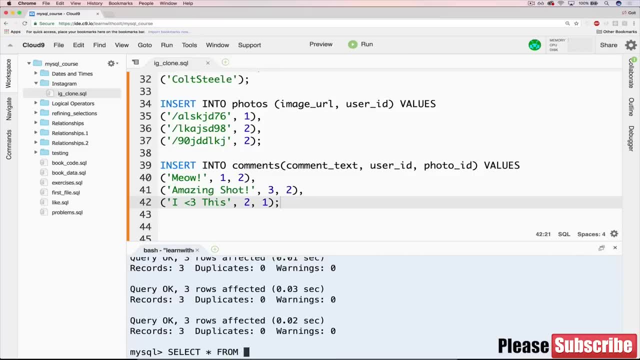 But we can do that now and make sure I have my semicolon instead of a comma there This time. if we source it, everything looks good. You can do a select star from comments. There we go. We've got three comments. 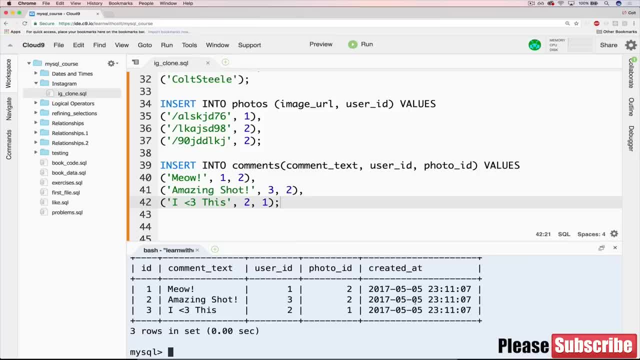 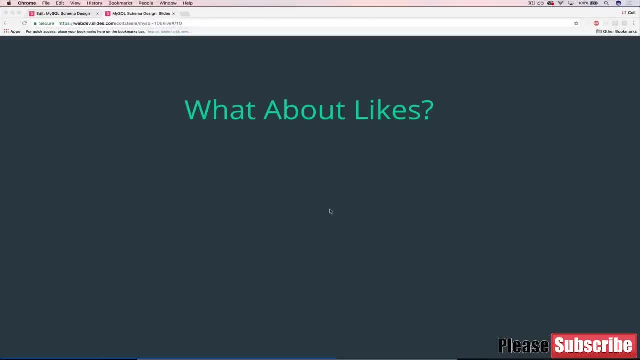 We could put a user ID in and a photo ID. I won't do that now. We'll do it as an exercise later with some more complex data. But of course you can do that if you want a little bit of practice, All right. 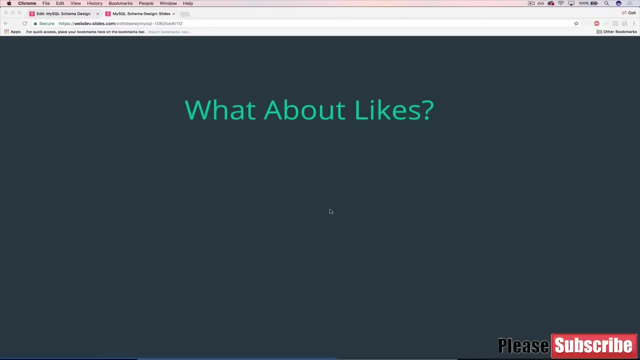 Moving on To likes. So we've seen now users, photos and comments and likes are a little bit similar. They are like the comments schema, because when we think about how likes work on Instagram, at least you like something. you like the particular photo. let's say it's corresponding to that photo. 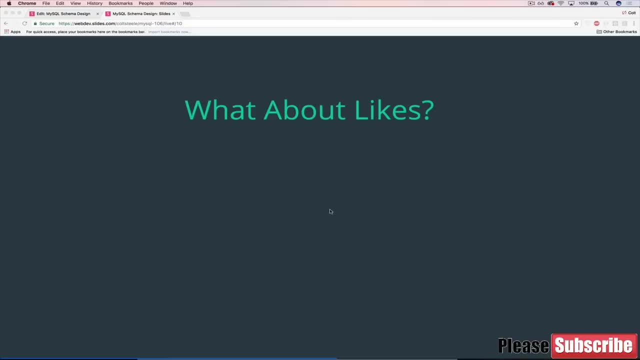 We need to have an association there. But then there's also the association between me, the person liking it and the like itself, And that might not matter if we allowed for infinite likes, You know, if anybody could like something as many times as they wanted. 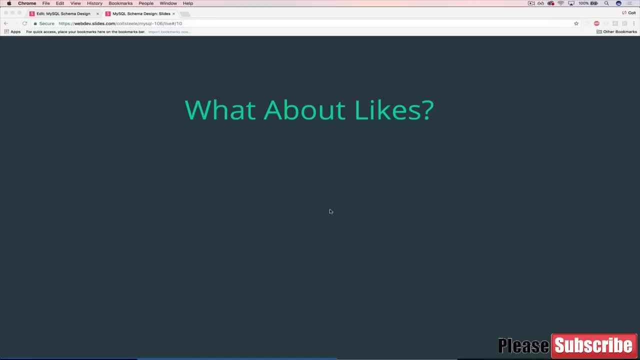 just it was a button that clicked and it just kept going Every time I clicked it. we could get away with not storing user information with a like, But even then it might be nice to see how many times somebody had liked something or how many likes you know I in general. how often do I click the like button? 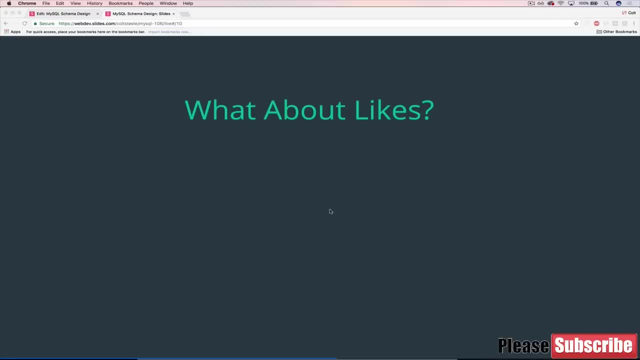 compared to somebody else. It might be. it might help us figure out who's a bot like on Instagram. That's a big problem. Actually, are these bots that people write, that go and just like photos, like things all the time, create comments that are just cookie cutter? 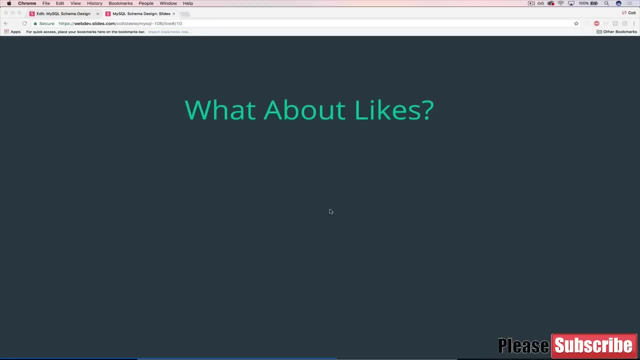 It's kind of frustrating actually, if you're a photographer, because you know you'll post something and then you get excited that you have, you know, one hundred people who liked it, And then it turns out a lot of them are bots. 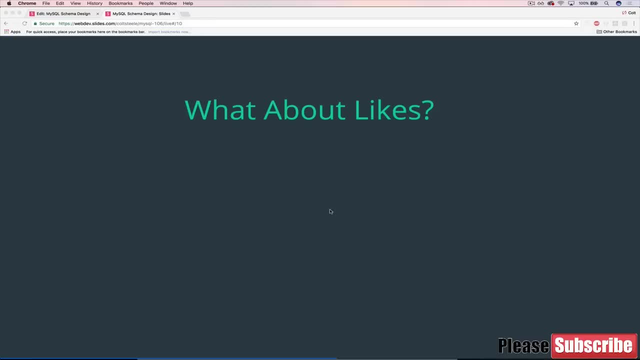 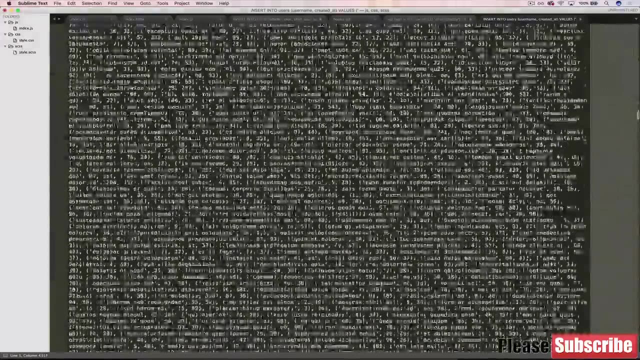 If you actually go, try and look at them, they don't have any photos posts. really, They always comment the same thing. Long story short, in this giant data set here, I actually coded in some bots that we'll be working with. 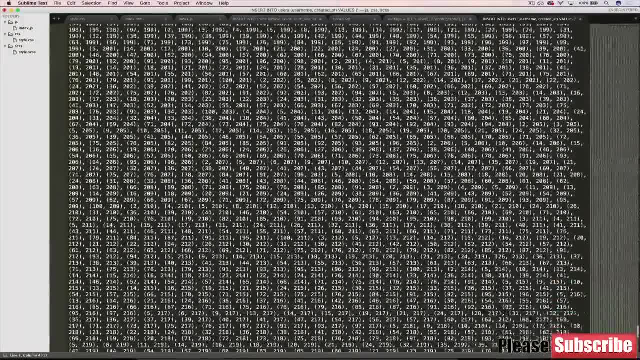 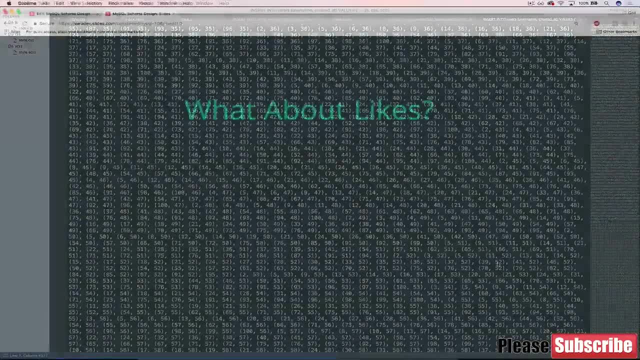 Basically people who aren't, who aren't creating much stuff, They're not posting many photos, but they are liking a lot of things and commenting the same thing a lot of the time. Anyway, back to likes. it's going to look like this: 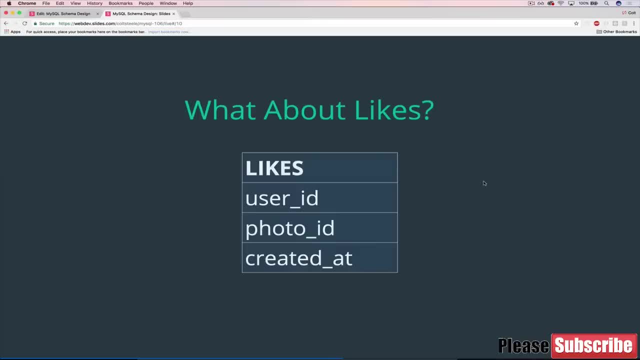 We'll have a user ID and a photo ID and a created app. So our user ID is going to refer to a user's ID and a photo ID refers to a photo ID And there's really nothing else. There's no information being stored there. 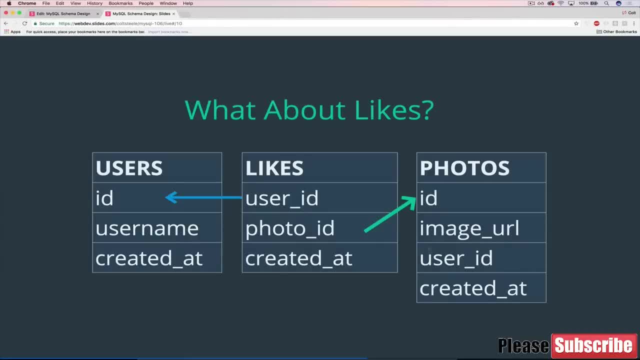 Maybe aside from the date or the time it was created when the like happened. But what else is there to store? You know, maybe Instagram is doing stuff like whether it was liked from the Web version versus the iOS version. Maybe they're storing, you know, other information here, possibly. 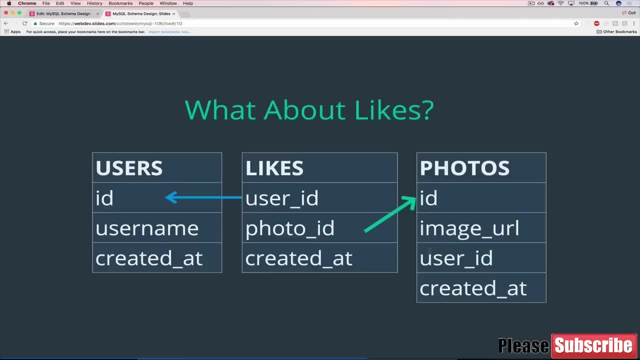 But for us this is the basics. We just need a user ID and a photo ID, And every time a photo is liked by a different user, we get a new like, just like this, with the user ID and photo ID. So we'll start by coding this: 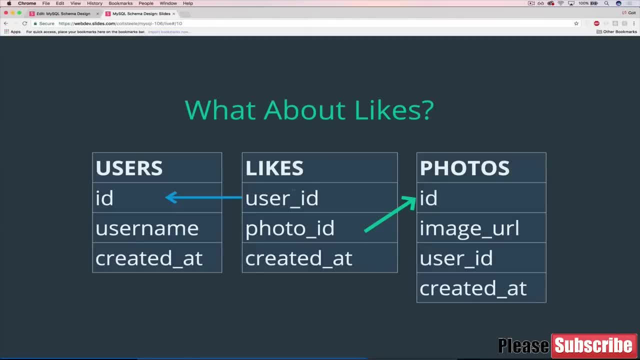 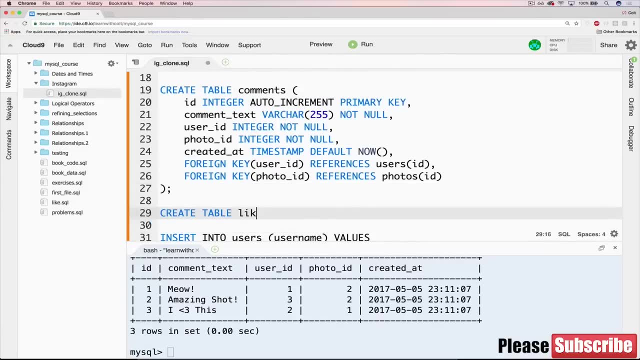 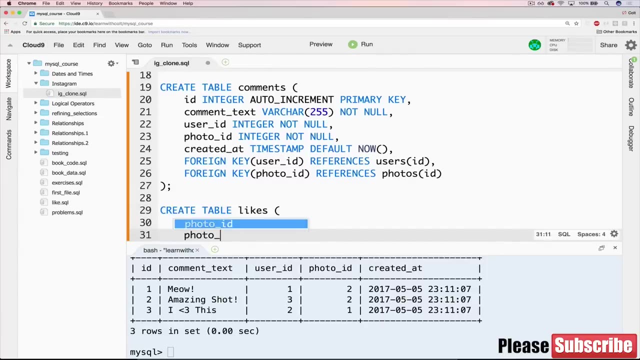 You might have noticed that I didn't add an ID to likes. I'll explain why in just a second. But let's start by creating our table. So we have create table likes and don't forget the semicolon. We have a user ID and a photo ID and are created at. 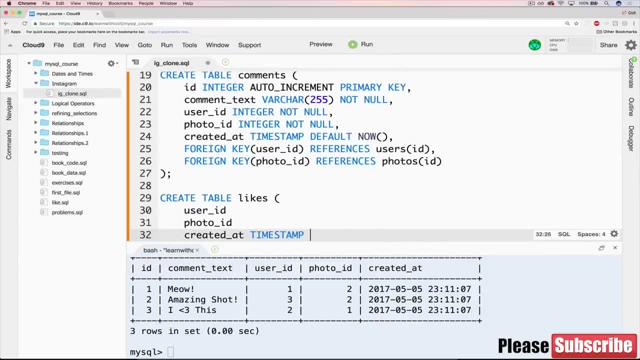 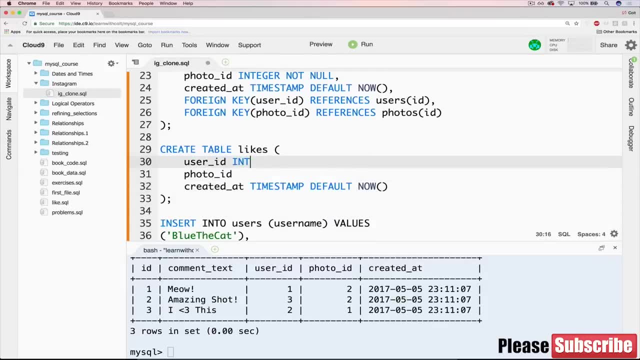 Let's start with created at. We often neglect it. Timestamp default now. OK, nice and easy. User ID is just an integer, Don't want it to be empty. Same thing for photo ID. But then we need to set up our foreign key constraints. 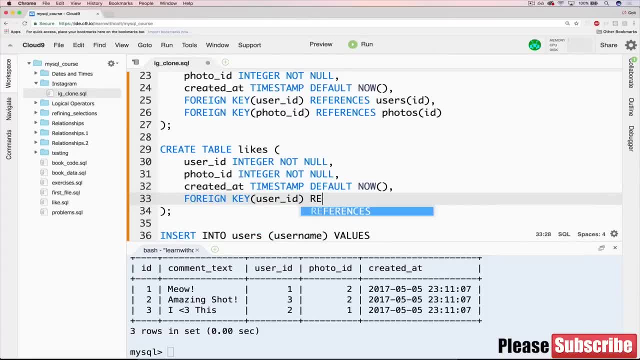 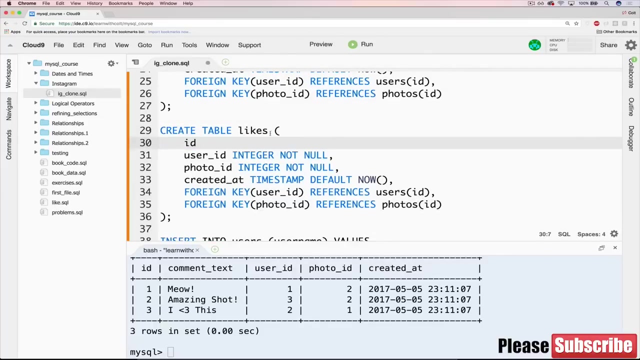 Foreign key: User ID References users ID comma. another foreign key, This time photo ID- References photos ID. OK, so now let's address why we don't have an ID here, And the main reason is that we don't need an ID. 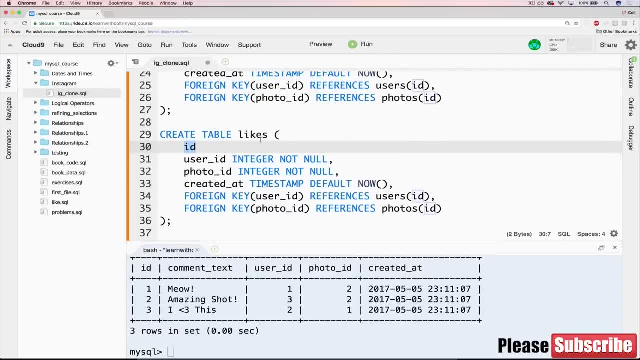 We're not going to be referring to likes anywhere else. If we were, it would be good to add an ID there, Maybe, but we're not having any table store information about likes. The other thing you might be wondering about is how do we ensure that there's? 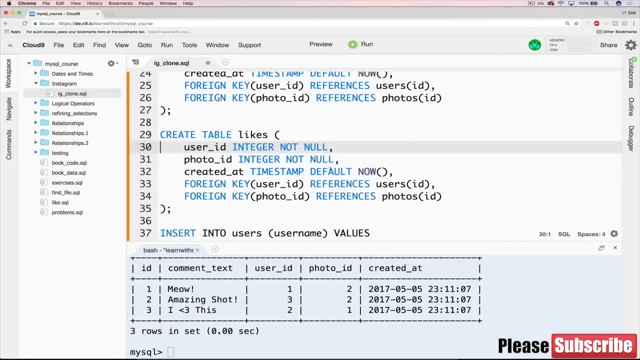 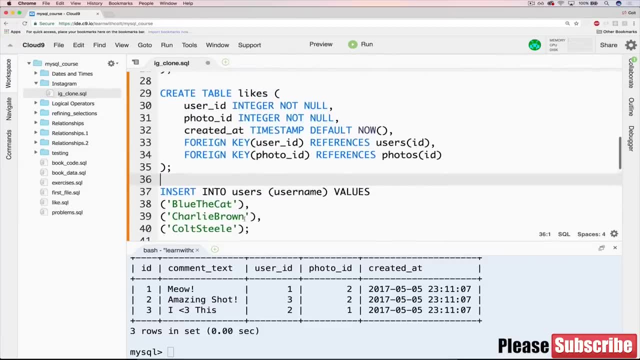 only one like per user is our way to do that in the database, Because right now, if I did this, I could just insert: Let's say, my user ID is one and a photo ID is one. I could insert a like with user ID one. 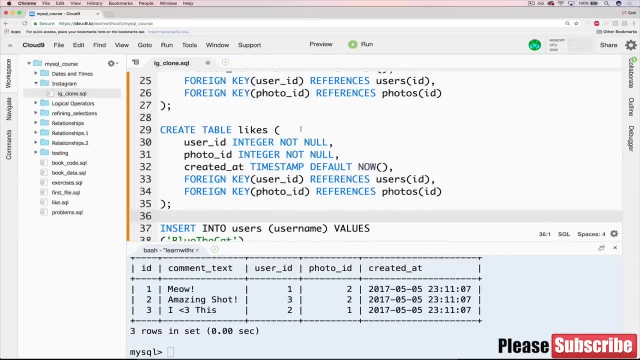 photo ID one and then insert it again and again, and again, And there's nothing stopping that. So what we really want to say is: we want a unique combination of the two. There can only be one instance of every combination, And there's actually a way of saying that we haven't seen it. 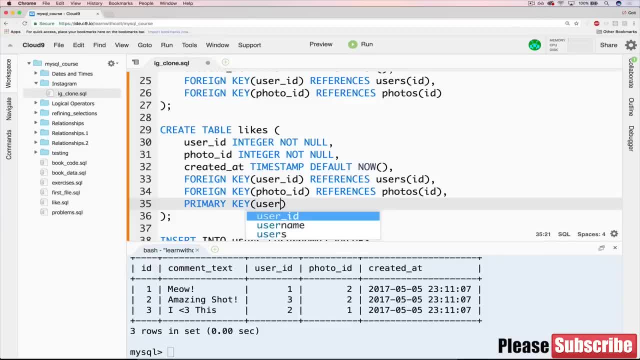 But you can do this primary key And then we can just say user ID, comma, Photo ID. So what this will do is basically not allow you to insert to likes that are exactly the same: the same user ID and the same photo ID. 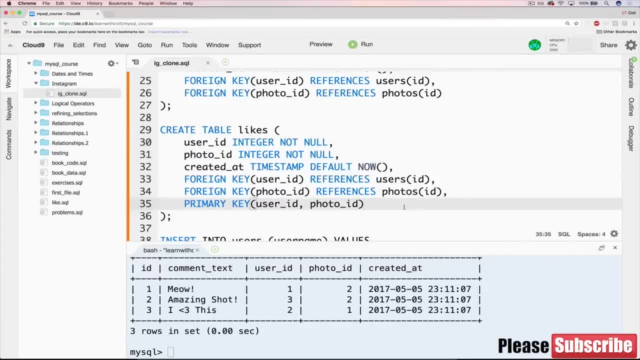 And I'll demonstrate that. if you feel confident, if you trust me there, you can skip, move on. We're done with the schema here. Let's just make sure that it runs. I don't have any syntax errors, of course. 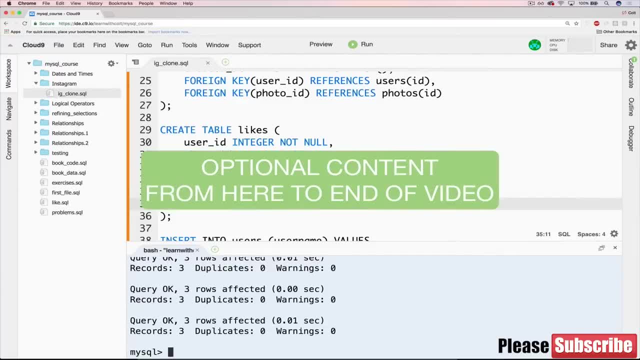 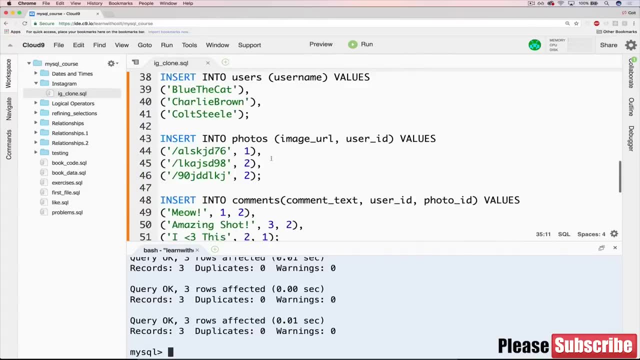 OK, it does, But if you like to see me try it out, like the last couple of videos, I'll do that now. So if you're still with me, all I'm going to do is take these photos in these users. 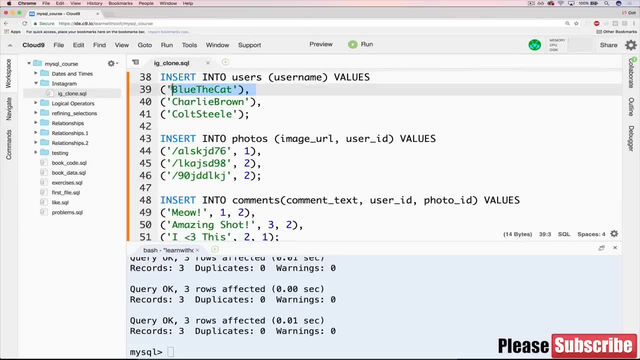 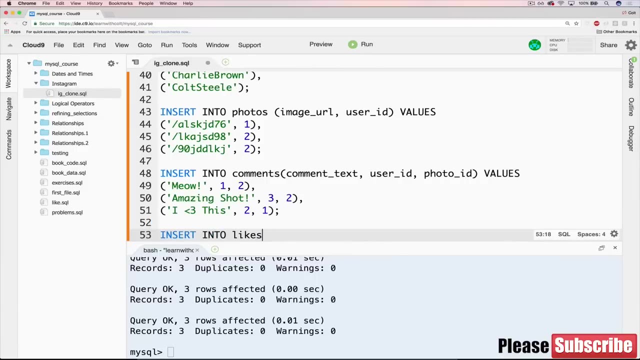 I'm going to have some of them like them. So let's take blue user ID one and that first photo. She created it. That doesn't matter, You can like your own photo on Instagram. So we'll insert into likes And we have user ID photo ID. 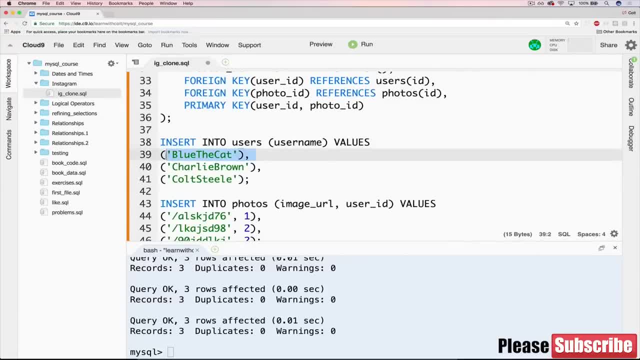 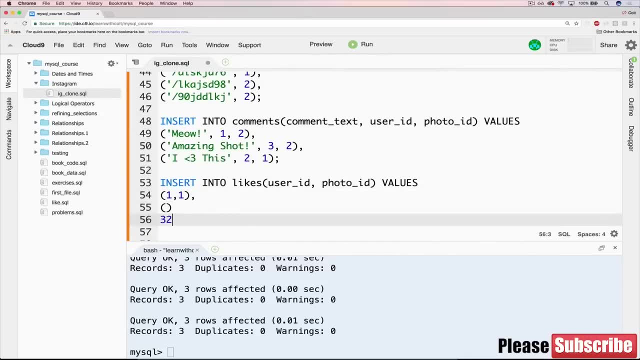 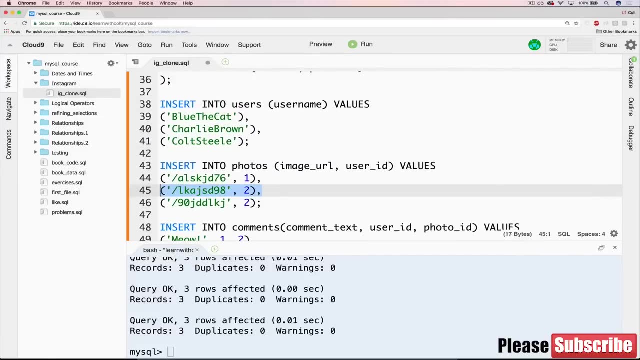 So the first one will be one comma one. So I'm inserting our blue is liking this photo, And then let's have Charlie Brown also like it, So that would be a whoops. Two comma one, And then we've got the next photo here. 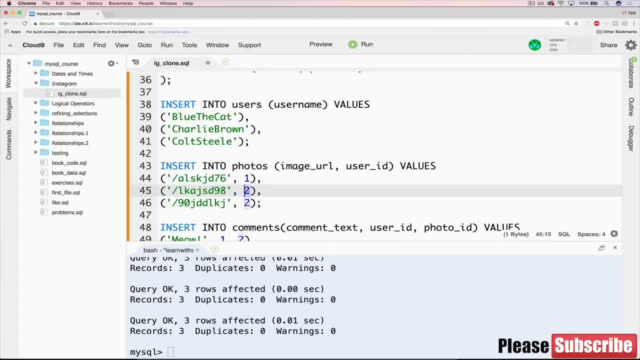 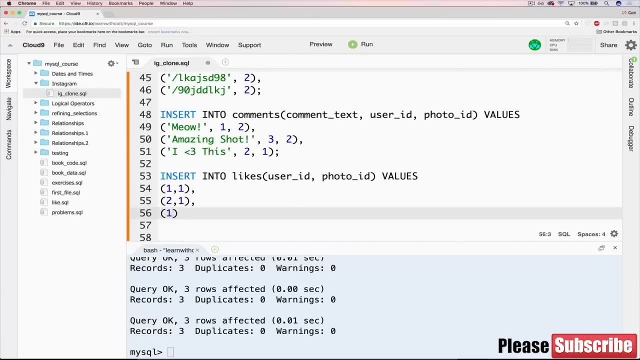 which has a photo ID of two, not this. Remember, this is the user ID who created it, But this has an ID of two. So let's say blue also likes that one. So blue ID of one likes photo ID of two and she likes photo ID of three. 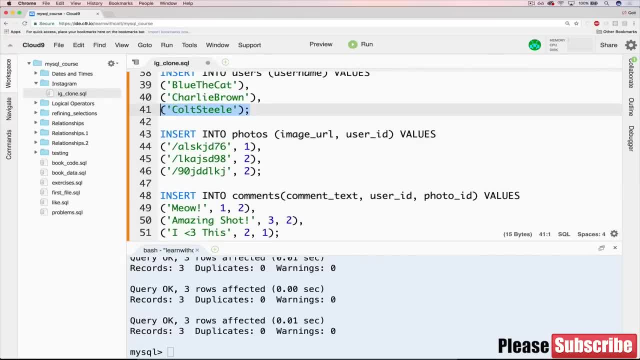 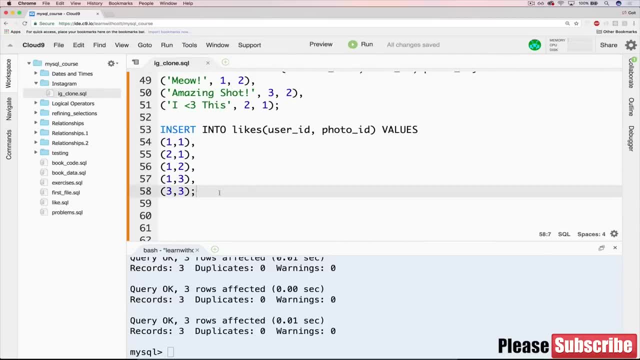 And then let's say I, I have user ID three. I like photo with ID of three. OK, so let's start there. We run it, It works. There shouldn't be any problems at this point. But now, if I try and do this, insert into 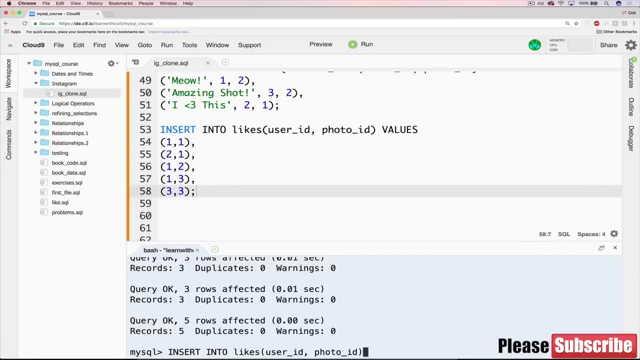 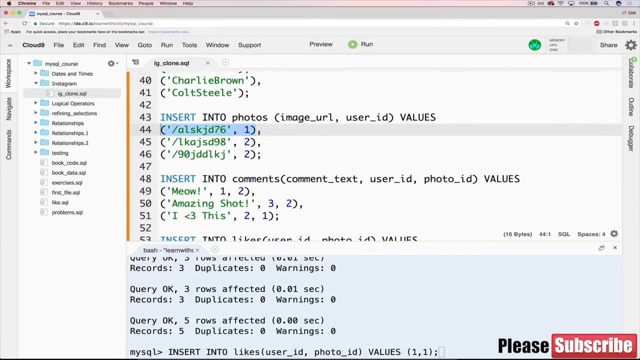 likes user ID, photo ID values, and I do one comma one. Well, that's not that, There we go. One comma one, which already is in there, Blue user ID one, And then this photo: Add blah, blah, blah 76.. 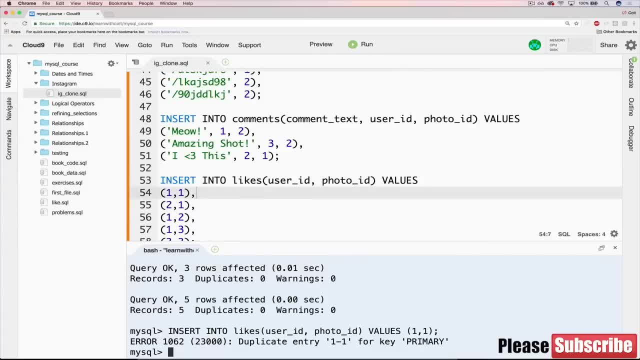 With ID of one. We already have that like. if I try it, you can see you get duplicate entry, one dash, one for key primary. So the way it does it is basically combined to to keep track of the combination like that, the dash between it. 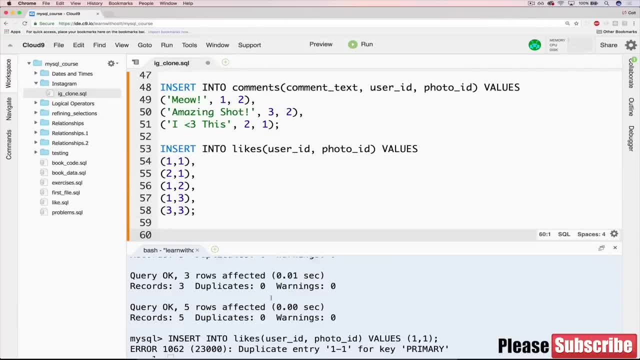 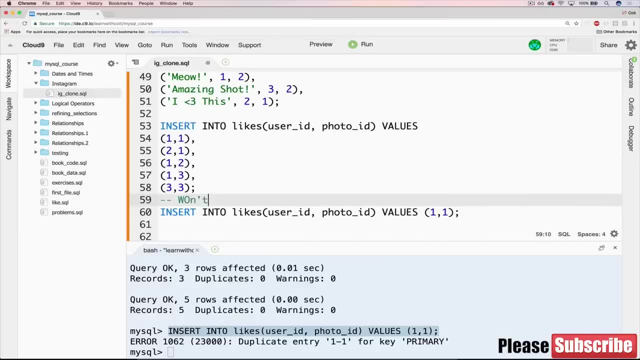 So that's pretty much it. I will copy what we just did and add a note here. If you're looking at these notes later just saying won't work because of primary key Constraint, and I'll comment it out as well. We don't want to run that every time, Great. 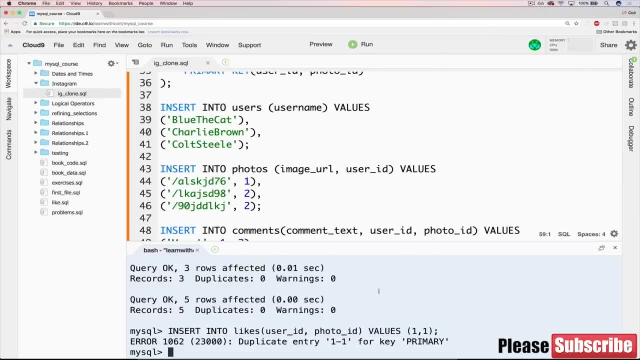 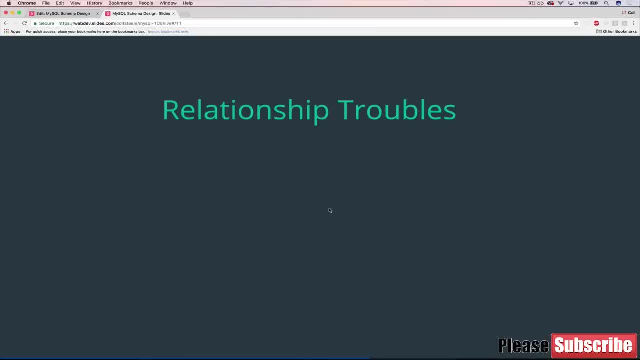 And next up, we're moving on to a fun one, which is relationships, following, followers, all that stuff. Welcome back. So we're moving on to capturing the relationships, the friendships between users. so we're talking about followers or followings, or however we want to term. 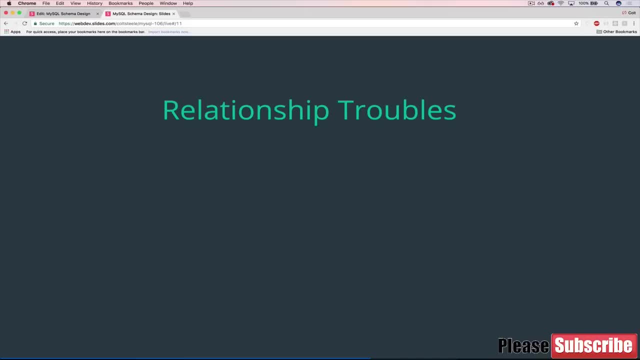 this. I just refer to it as follows, but it's not really a great term Either. But basically, how do we capture the data when I follow another user and they may or may not following back, it doesn't matter, I'm still able to follow them. 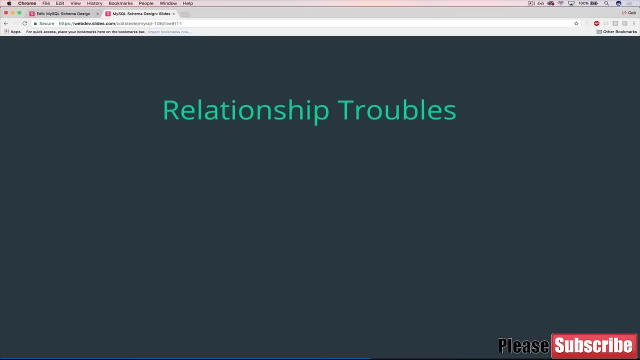 And that's all we need to capture is this one way relationship, And the easiest way to do it is with a single table that will call follows And all that it is is two user IDs. So both of these are primary. Excuse me, Both of them are foreign keys referring to a user ID. 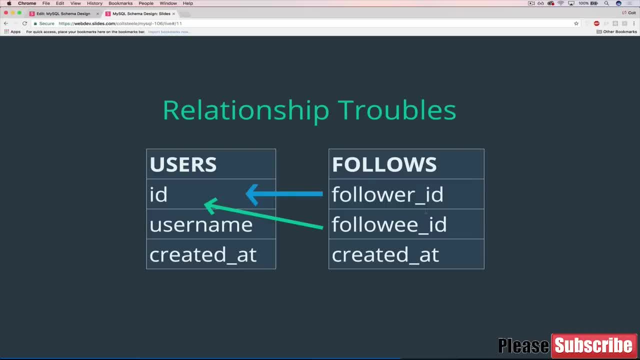 A different user ID. That's important. We can't have a user follow him or herself, So there are different IDs and I called them follower ID and follow ID. You could do user one ID and user two ID, But the idea here is that you can tell who is following who. that the follower. 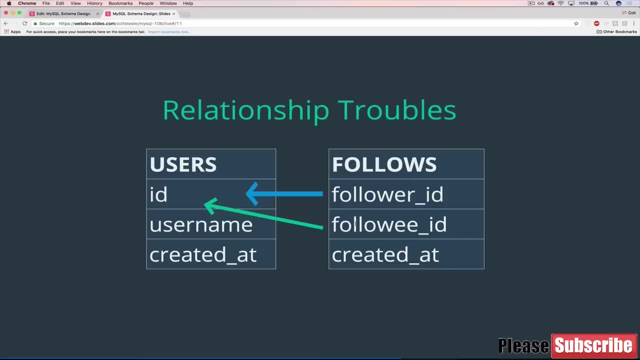 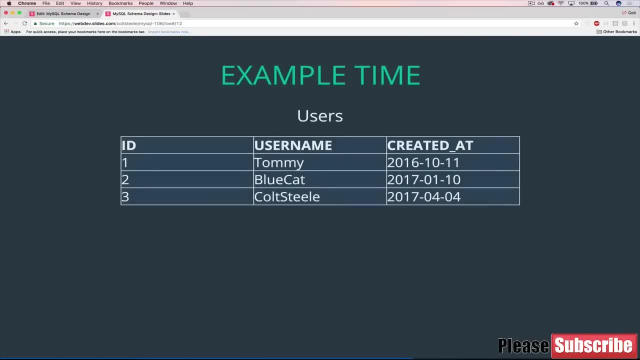 is the person following the follow- we. it's a nightmare to try and discuss here, So let me give you an example. Here's our table of users. So we have three users- Tommy, Blue Cat and Cold Steel- And they have an ID of one, two and three respectively. 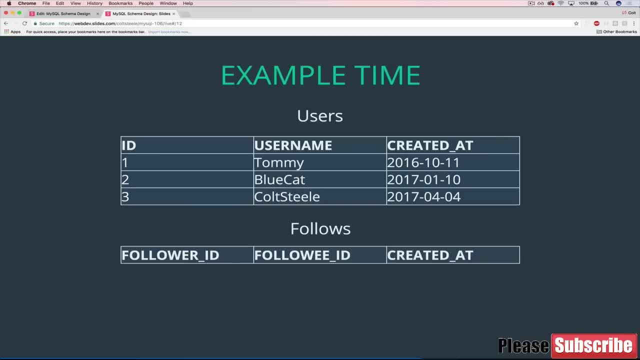 OK, so here's our follows table, And the first thing let's say that Colt me decides to follow blue. So that means you know follower ID is three, follower being me the follower. Who am I following to blue? the following: 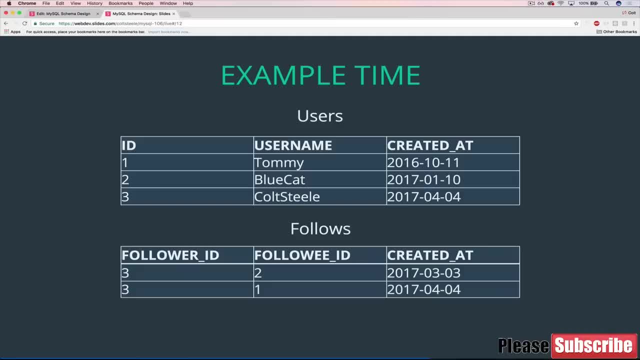 But she doesn't have to follow me back, and she doesn't follow me back, At least not yet. If you look next, I'm following user ID of one, which is Tommy Speaking of blue. Yes, OK, let's see where was I. 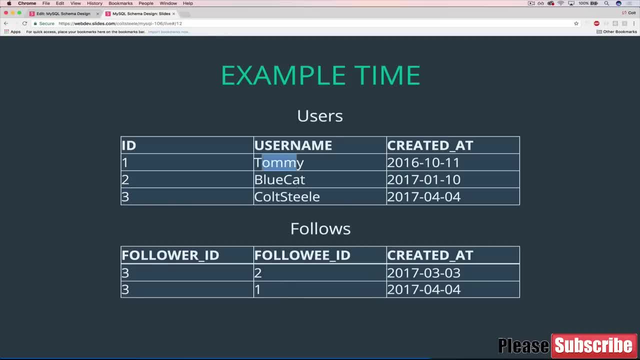 So I was user ID three: follow Tommy. OK, And then you can see now blue is user ID- is to finally follows me back. She decides I'm a good owner and she wants to follow me on Instagram. But the key thing Here is that it's a one way relationship. 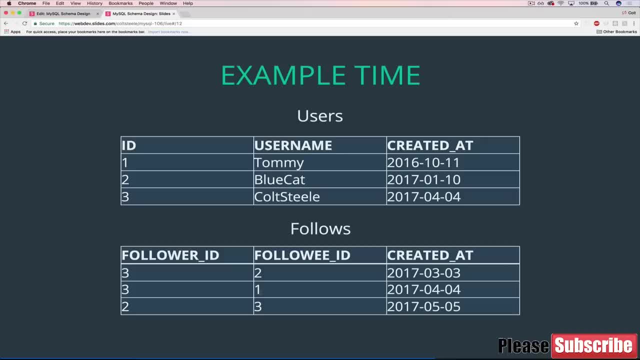 You know, here we have- I'm following Tommy, but Tommy does not follow me, And this is all. we need the structure to encode that information. A couple of points we should make: that these are both foreign keys created at. It's just good to know. 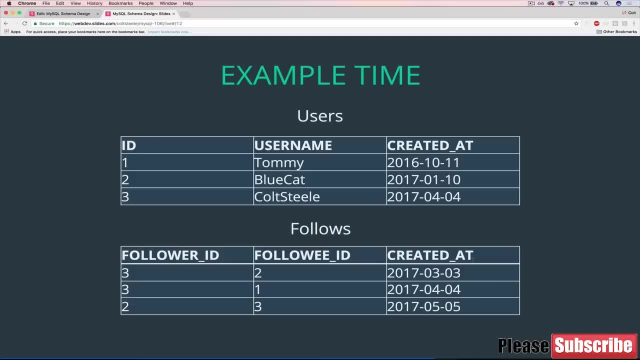 if you want to keep track of, you know when people are being followed- Again, not essential, but something that Instagram definitely is tracking. you know friendship date or something, And then also, we don't want to have duplicated you know follows. 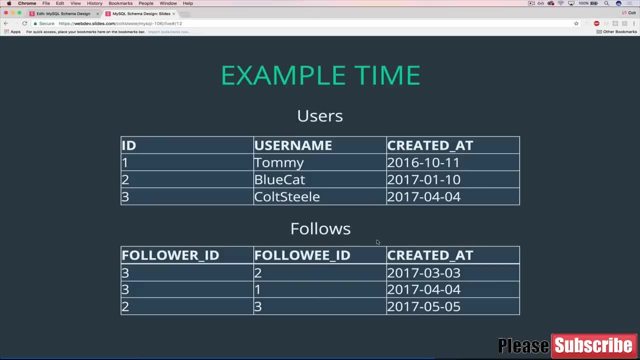 So I don't want to be able to follow blue again. So we need to enforce that These are unique, The combination of these two in an order. So, as you can see, you know, three and two is here and we can't have two and three. 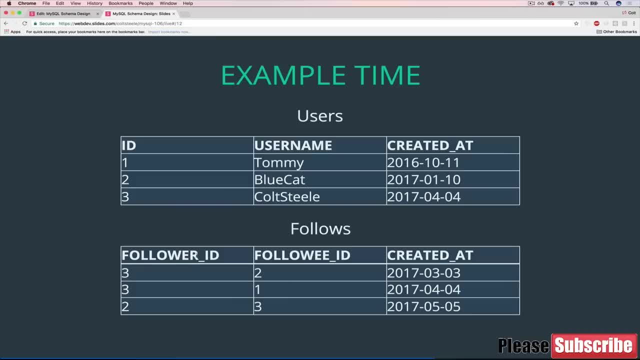 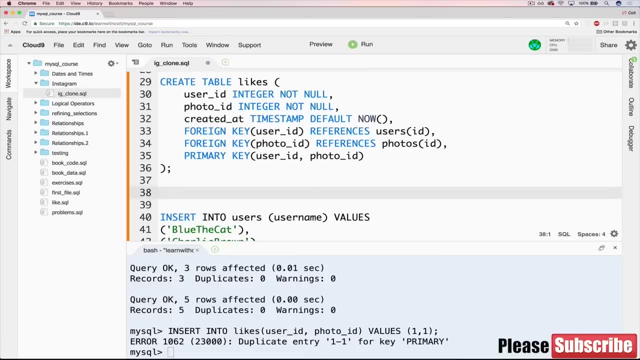 but we can't have another three and two. OK, so let's get to it. I've got follow ID, follow ID and created at and we won't be needing a primary key ID or an ID integer. that is a primary key because we won't be referencing. 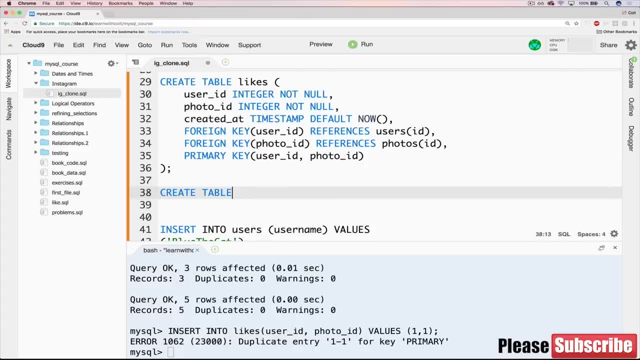 these friendships or follows anywhere. So create table follows. If you have a better name, feel free to use that- And the first thing we have is our follower ID and our follow E ID and then create that. OK, oh my gosh, OK. 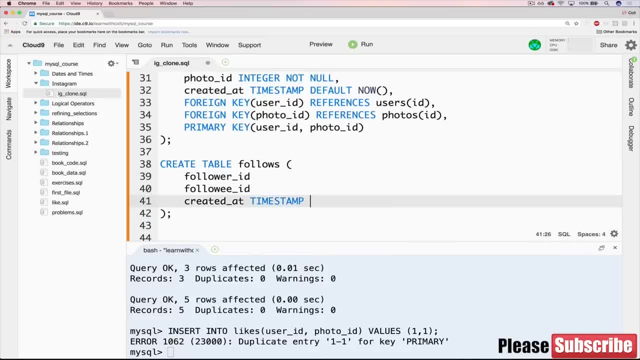 So let's start with created at timestamp default now. Perfect. Then we've got follower ID and follow. E and D are both integers. We don't want them to be null. Copy that on over our commas there. And now we also need to officially declare these as foreign keys. 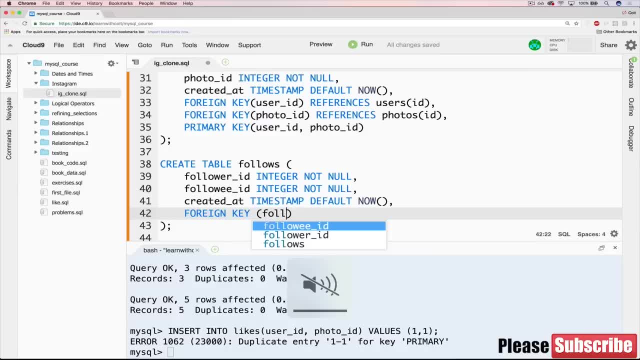 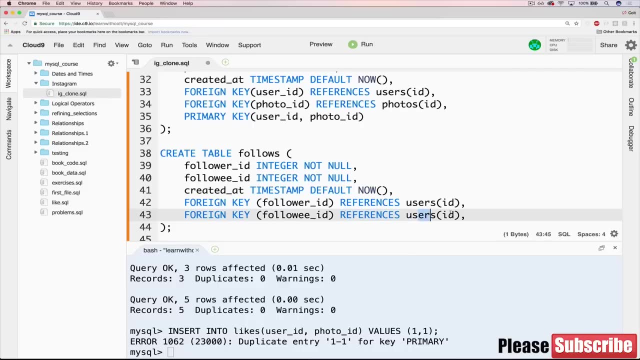 So that would be foreign key. follower ID references user users ID And we can just duplicate Copy that line and just change follow E ID. It also references users ID. And then the last thing, as I mentioned, is we want to enforce that you can only have one of a given relationship. 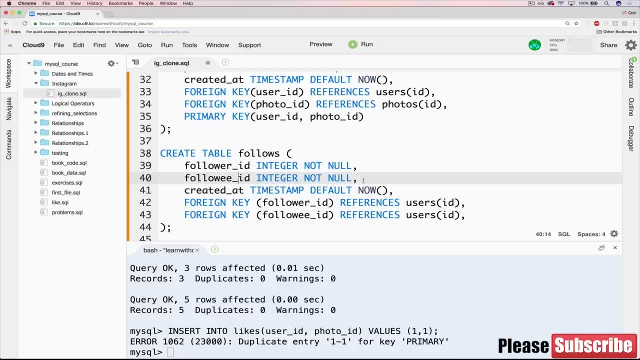 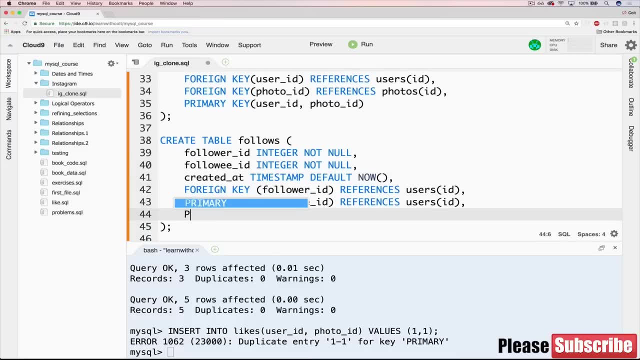 So if user ID one is following user ID two, that cannot, but that can only be in the database once. But user ID two can follow user ID one Anyway. so to do that it's just a matter of primary key in the order. that we actually put them in here won't really matter. 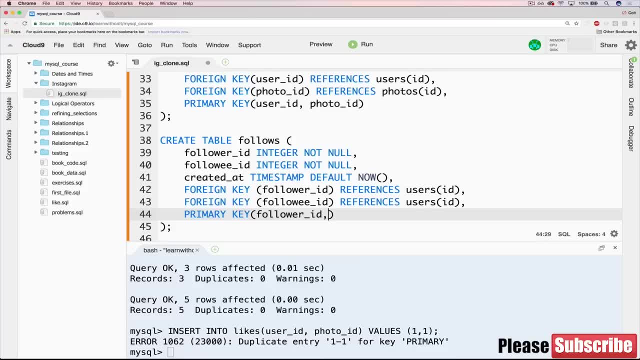 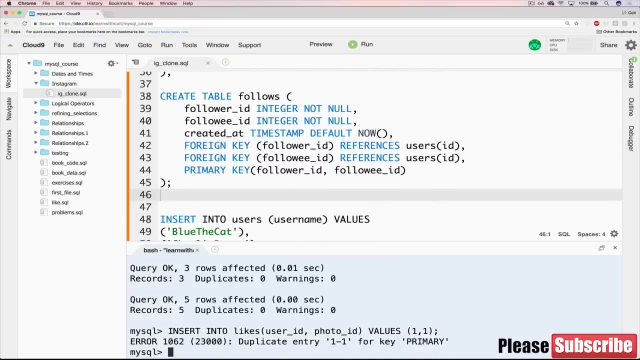 I mean it makes a difference to my QL, but for us it won't matter. Follow ID: OK, so that creates the table for us. Let's just check that everything works Looks good. Let's do a describe follows. 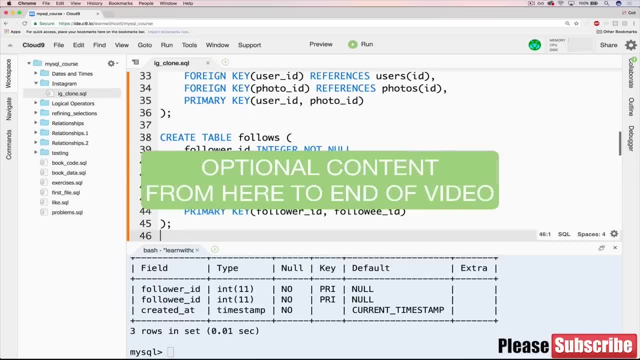 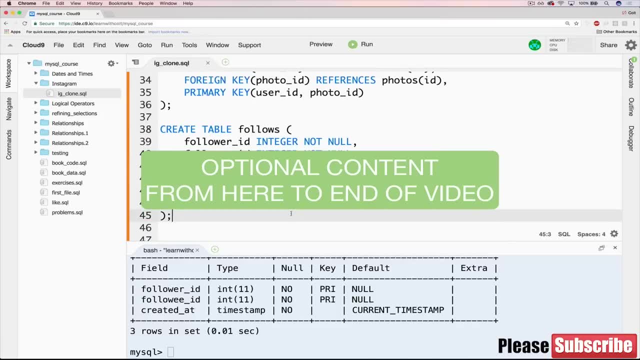 Good, All right. So, just like the last couple of videos, we're done. If you want, stick around and I'll play around with some data and show you that this primary key constraint is working. OK, so if you're still here, 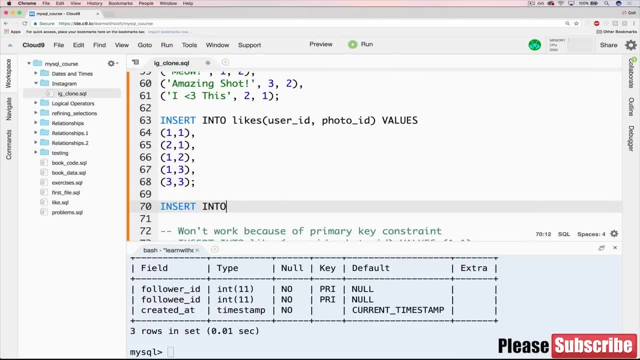 let's try doing an insert into follows and we'll have our follower ID first and then our follow. we ID Gosh. it starts to just sound like gibberish after saying it enough times, So let's say that we start off. We've got these three users right. 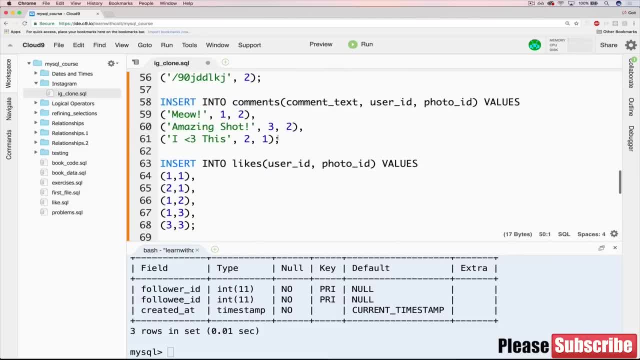 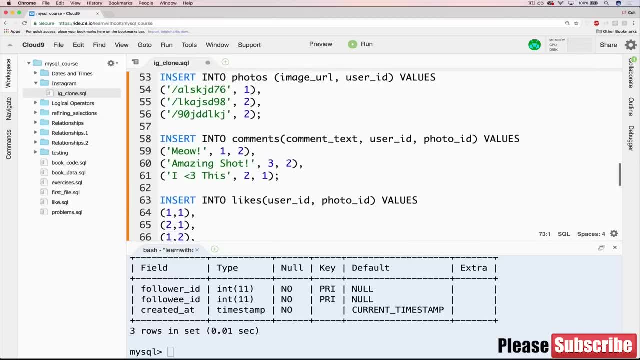 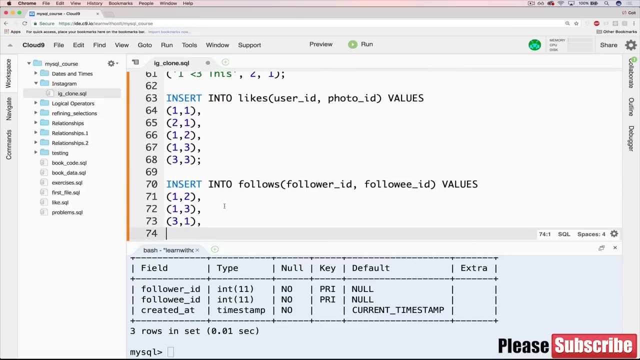 So blue Follows Charlie Brown, So that's going to be one common to, And we'll also have blue Follow me. That's one comma three. And then let's say I also follow blue back, So that is three comma one. 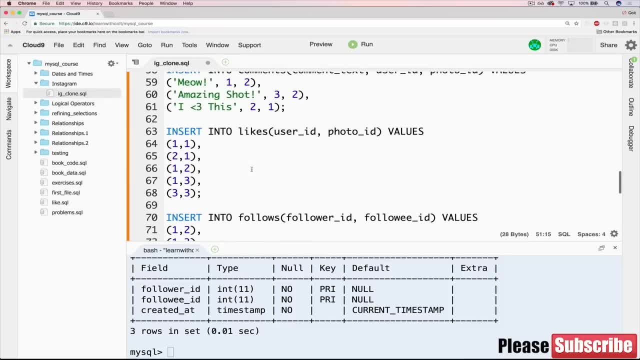 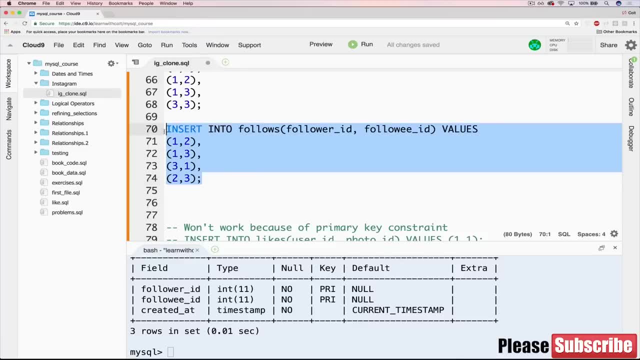 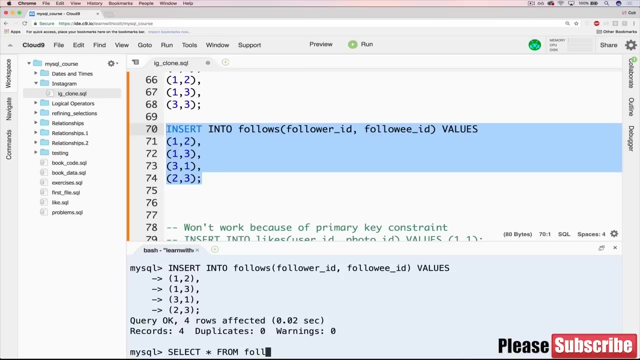 And then let's say that we have Charlie Brown follows blue. Let's say: Charlie Brown follows me. So that's two comma three. OK, Let's try inserting them. Looks like it works. You can do, you know. select star from users. excuse me from follows. 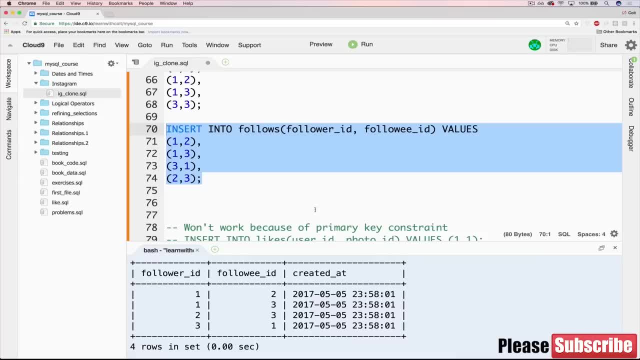 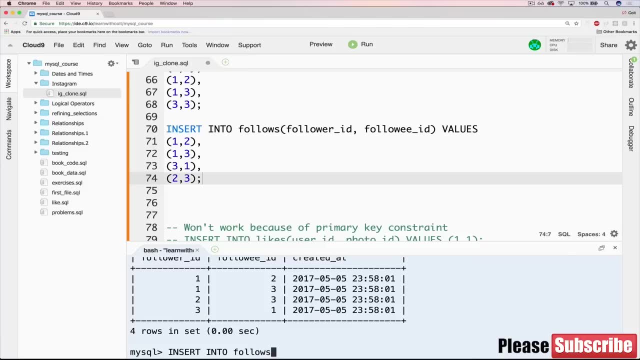 Great, We got follower ID, follow we ID and created that. And then the true test is if I try and re insert a relationship like insert into follows, getting sick of this follower ID, follow we stuff. We're almost done. So let's say, try and insert this friendship one comma two. 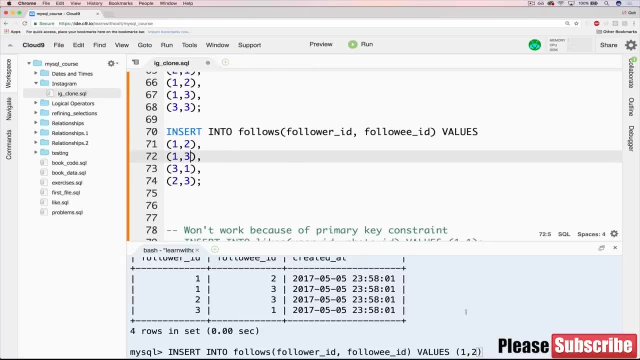 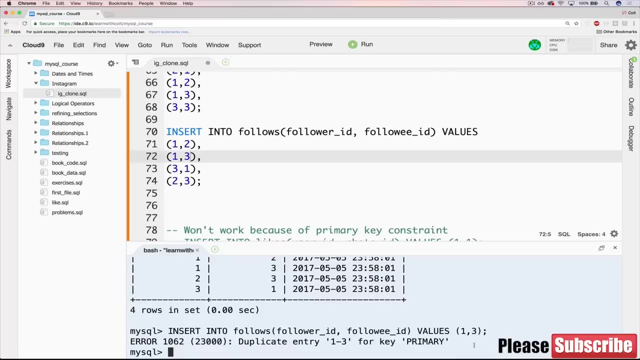 So that is blue following. Let's do one comma three. It's blue following me. She loves me so much She wants to follow me again. If we try and do that, it's a duplicate entry. But as we saw, you can see here we already have three comma one. 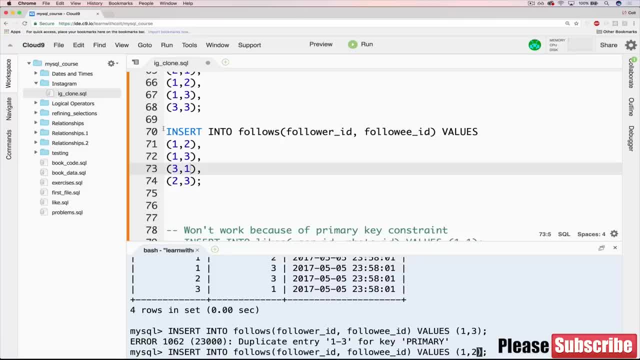 So if I did do, if I do one comma two this time, which we also already have- it's blue following Charlie Brown, It's a duplicate entry. But if I switch the order and do two comma one, that's permitted because we don't have that in here yet. 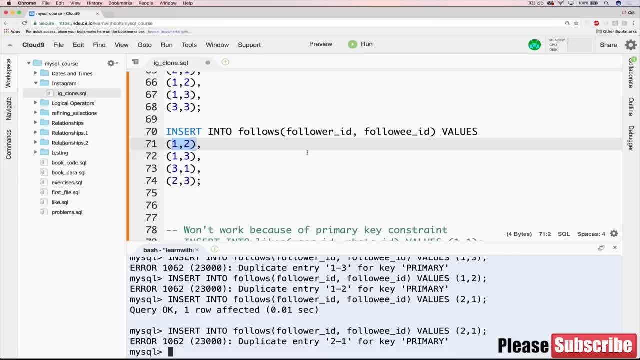 But now, of course, it's duplicate entry, So the order does matter, right. So who's following who? OK, so hopefully that makes sense. We're moving on now to our final piece, which is tags, hashtags, And finally, we've arrived at our last. 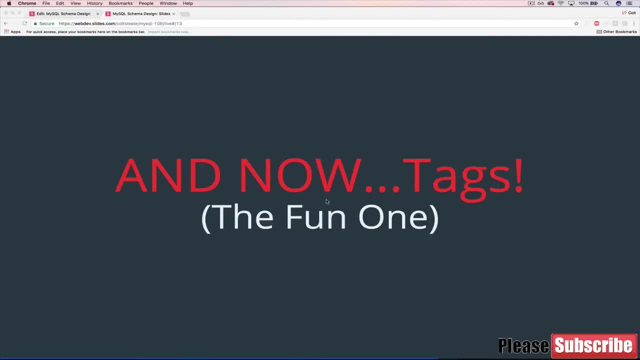 entity to store, which is hashtags or tags, And we save this one for last because, as I mentioned in the intro video, it's the hardest, I guess. Well, it doesn't have to be, but there's a couple of different solutions we could. 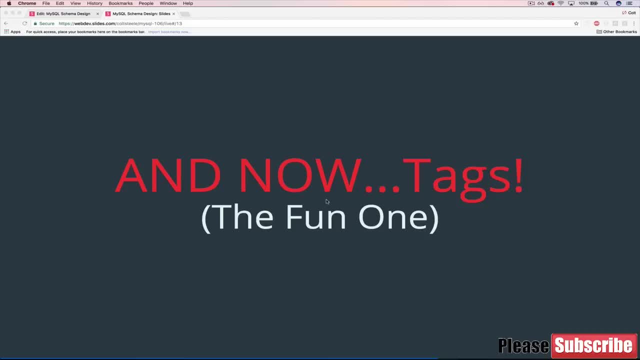 go about, and I wanted to have a discussion about which is best if there is one answer. So let's step through Three potential structures that we could use And remember. the way that this works is that one photo can have, you know, 10,, 20,, 50 hashtags. 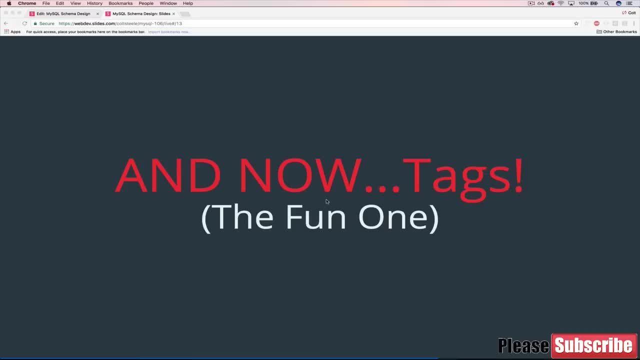 I do think there is a limit on Instagram. I mean, you can keep adding them as many as you want, but only 30,, I believe, actually will show up, or it's not that they won't show up, But it's that when you search for a hashtag, your photo will only show up. 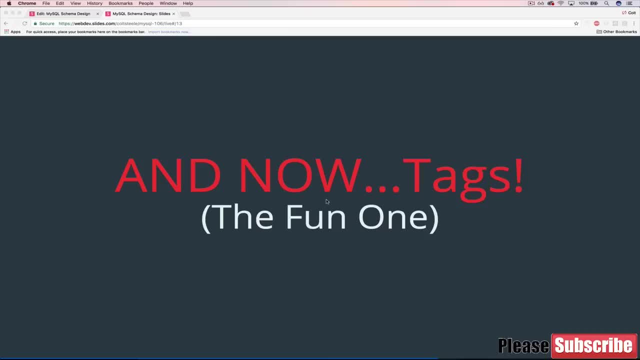 if you use less than 30. anyways, we're getting off track here. But the idea is, you, You can add hashtags to a photo, but then you can also, you know, go click on a hashtag and see all the associated photos with it. 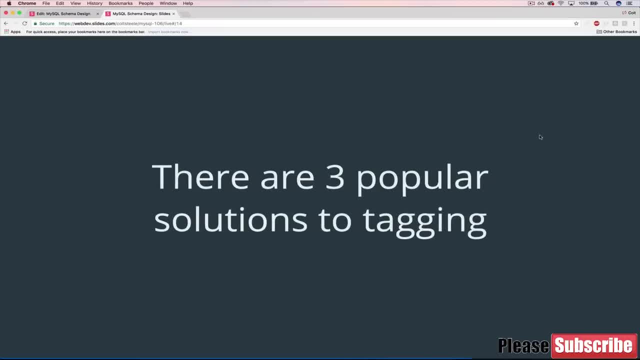 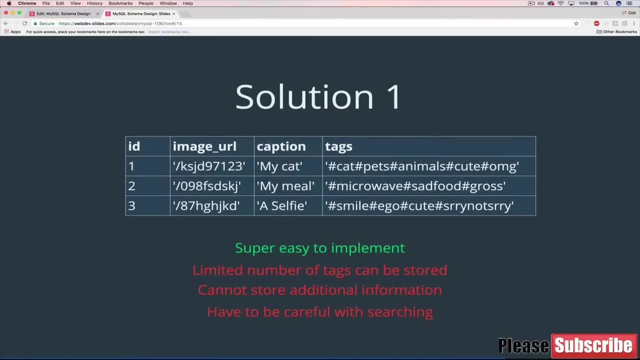 So here's one way we could structure it, which might seem maybe the least obvious to you, which would be to do it like this, where we actually just have our photos table, But we add a column called tags, and it's a string. 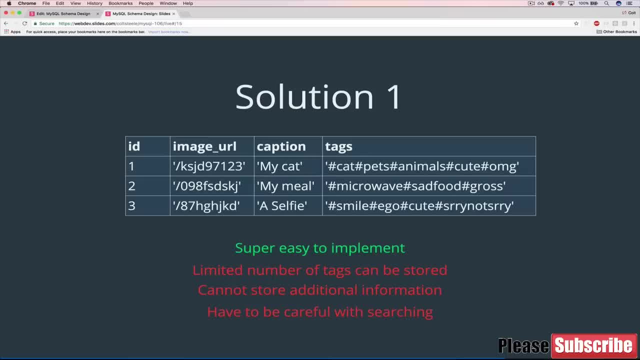 It's a varchar that just has our tags and we could separate them by the hash sign, the octothorpe, or by space- It is or dashes or something- but we're just storing them together And this could work in places to use this. 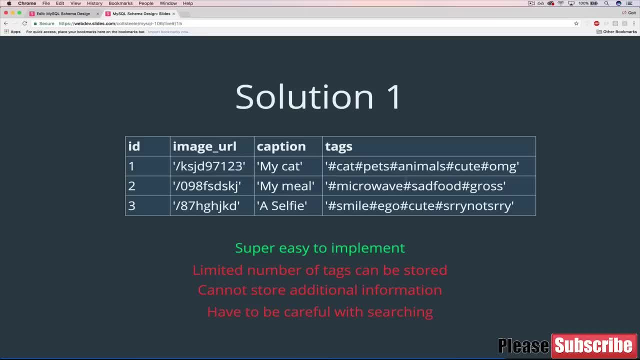 I've seen it suggested. at least I haven't seen it in practice, but you can imagine how it would work to add a new tag into something. You'd basically just take all the other tags and then concatenate in at the end a new tech or at the beginning. 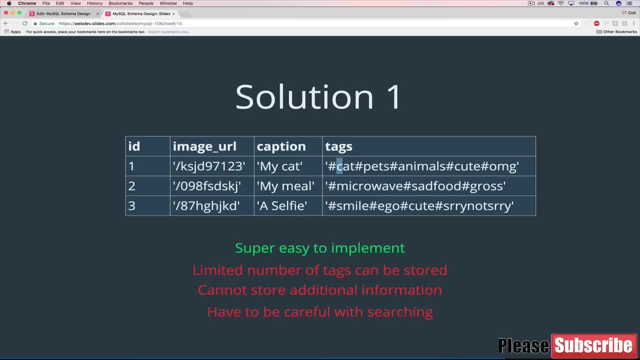 And then you could have an order to figure out which ones were posted first, I guess, based off of that order that they're in. And it's pretty simple, You know, if you wanted to find all photos that are tagged with cute. 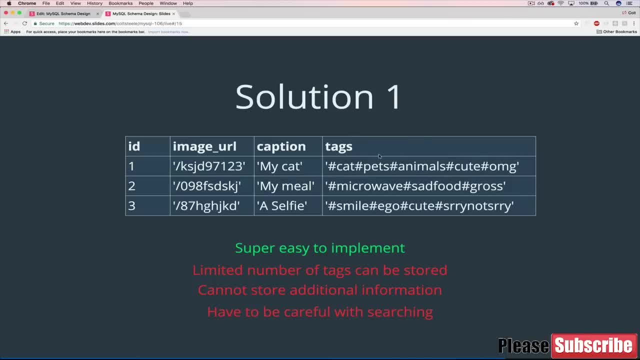 you just basically have to use like Where tags, like cute. But then, as you can see down here, there are a couple problems. Let's start with an advantage, which is that it's very easy to implement. You don't need any other tables. but there are a couple of disadvantages. 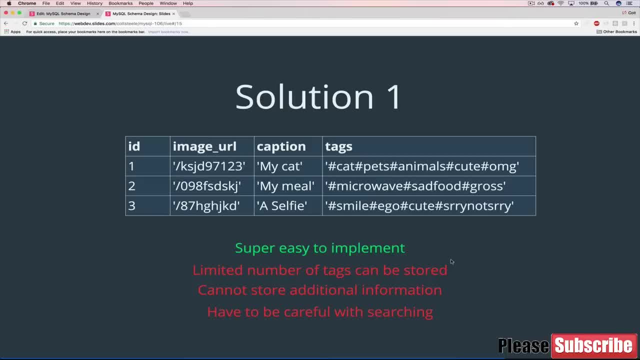 One is that there's a limit to how many tags you can have in there, which is the length of whatever the column is of a varchar. whatever the maximum length is, There's no money in there. The other problem, or another problem actually- is that you can't store. 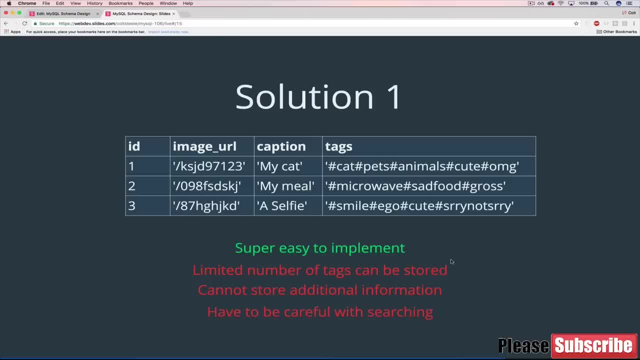 additional information. like you know, if we wanted to store the first time a hashtag was used, if I wanted to be able to see the first person to use the hashtag- whatever- cat or something- I'm not storing the time that something was tagged, because you know. 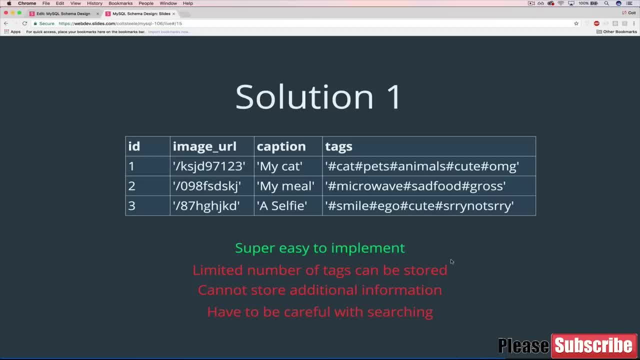 on Instagram you can add hashtags after the fact. I'm sure they're storing that when they're tagged so that they can track trends as hashtags come and go. It doesn't allow us to store additional information like that. And then the other thing that's kind of important is that you have to be careful. 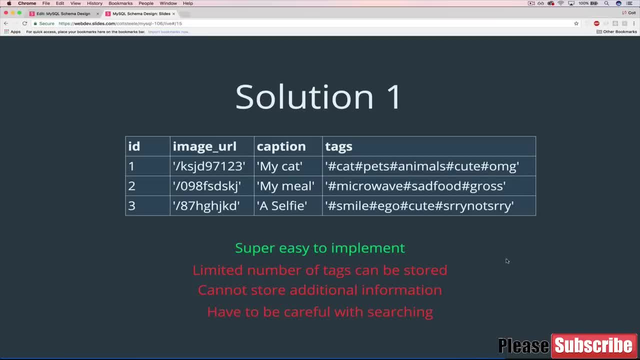 when you're searching for stuff. So if I was trying to find the hashtag food and I wanted to see nice food, beautiful food, So the hashtag is just food, Well, it will return this, which has sad food if I'm just doing like food. 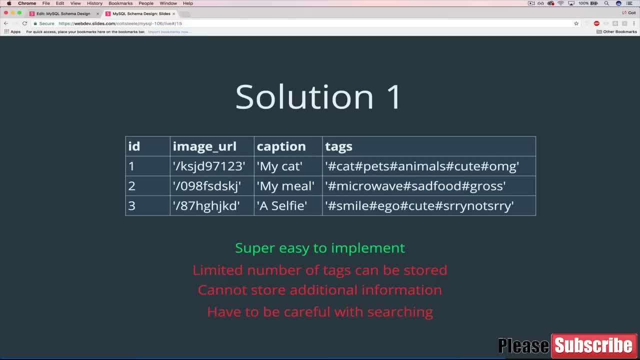 So I'd have to be careful and I need to add spaces, maybe to make it easier to separate things out. Basically, you just have to be careful in those ways around it. We've seen them before how you used search with like, But the point is, this is an easy solution. 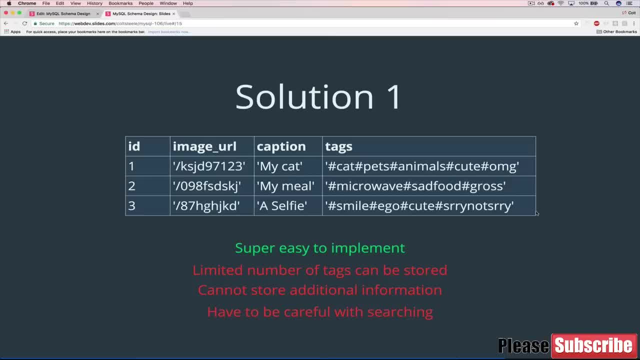 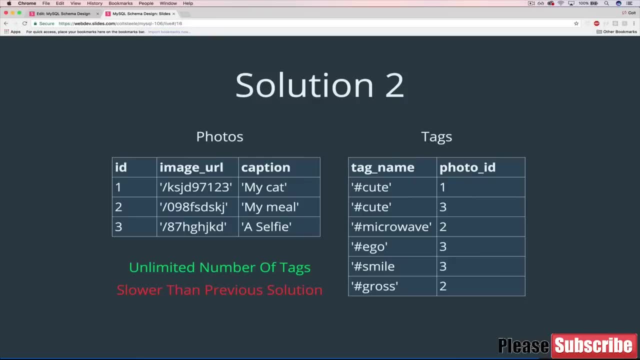 but it's not going to be the best and it's not the best for us right now. So another solution is to use two tables. So we have our photos, as our photos table currently is now, But then we have a tags table where we have our tag name. 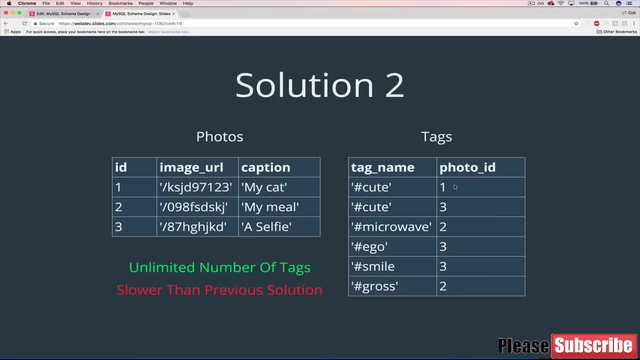 in this case cute, and then a corresponding photo ID. So you know, if this photo with ID of one is tags cute, we put it there. And then a photo with ID three, which is the selfie here, is also tags cute. 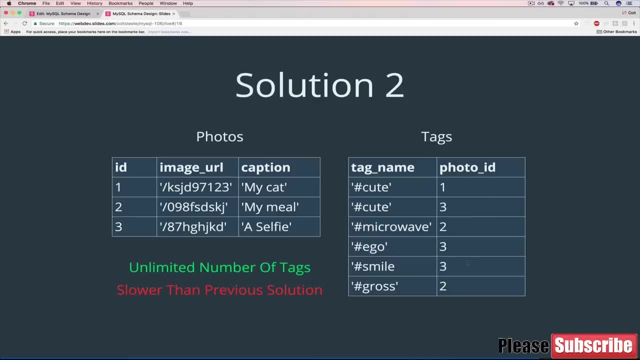 And then photo ID two is tagged with microwave and three with ego, three with smile, two with gross. So, as you can see, we can have a single photo with multiple tags, like here where we have this selfie. ID Three is tagged with smile, ego and cute. 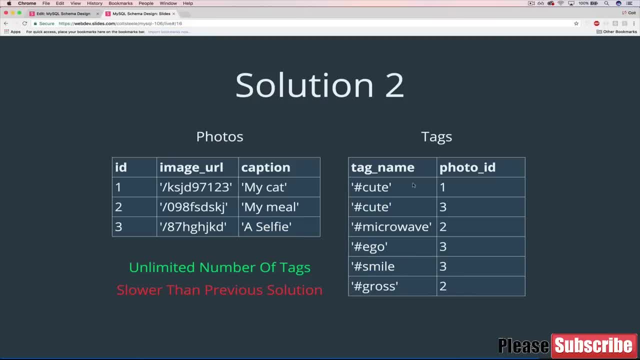 And we can also have tags that are applied to multiple photos, like cute. It's applied to the first photo and the third photo, So this works. There's unlimited number of tags. You know, that's an advantage. We don't have to worry about how many can fit into the string. 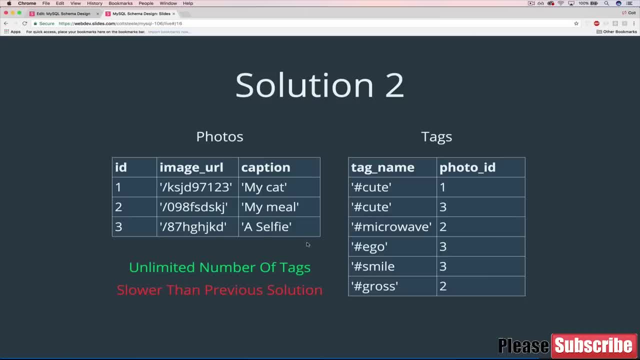 But a disadvantage is that, for one thing, we are storing, you know, these tag names over and over and over and these are strings, and that it's maybe not ideal to store all these different strings and have duplicated data, But it's not a big deal. 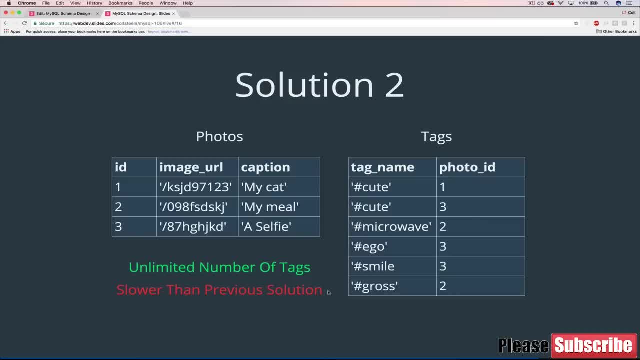 The duplication isn't the problem. Really, what it comes down to is that this is actually slower than the previous solution when it comes to things like inserting or updating or deleting, But then another problem is that it's actually slower than the previous solution. 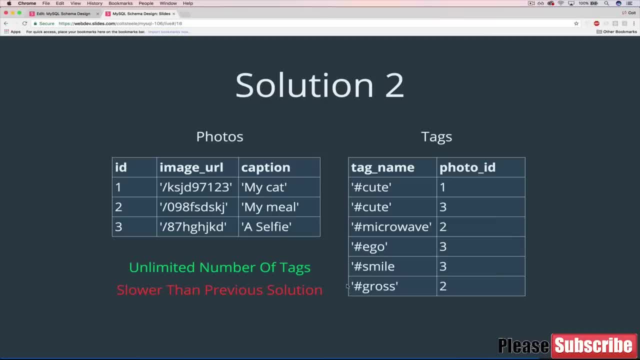 So in just a moment I can show you a comparison that I didn't do, But there's a great article that I found where somebody does a speed test between these, the three solutions, to figure out when they perform best. So this is not one we're going to use either. 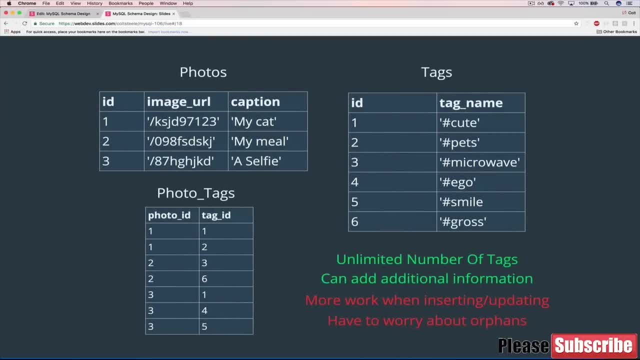 But solution three is, which maybe you've got It- involves three tables. So we have our photos table unchanged. We have a different tags table. So this tags table is just a tag name and an ID. And then we have a middle table, a joint table called photo tags or tag. 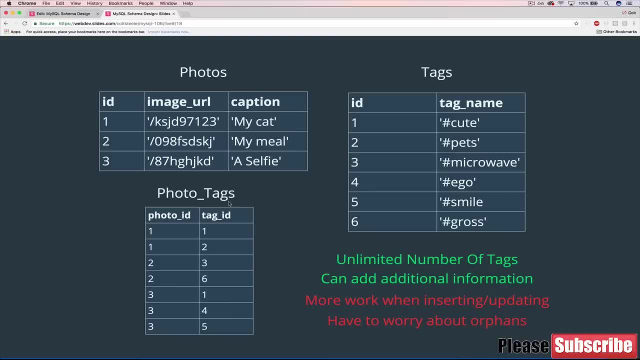 photos, or tagging or something- whatever you want to call it- which is an instance of a hashtag being applied to a photo, And all that it is is a photo ID and a tag ID, And that's it. So In this case, you know, photo ID one is my cat. 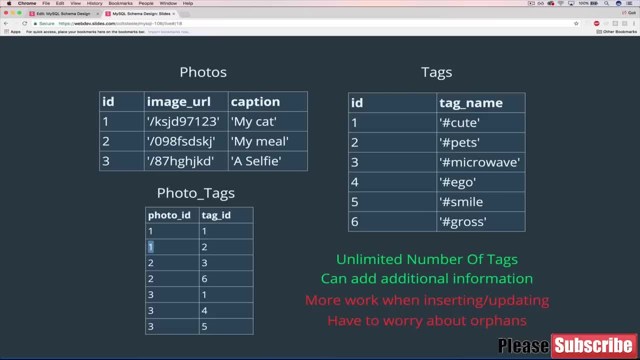 Is being tagged with cute, and then the same photo, my cat- is being tagged with pets, and then we have- we can keep going- my meal is being tagged with microwave and my meal is being tagged with gross, and so on. So we have these two columns and that's pretty much it. 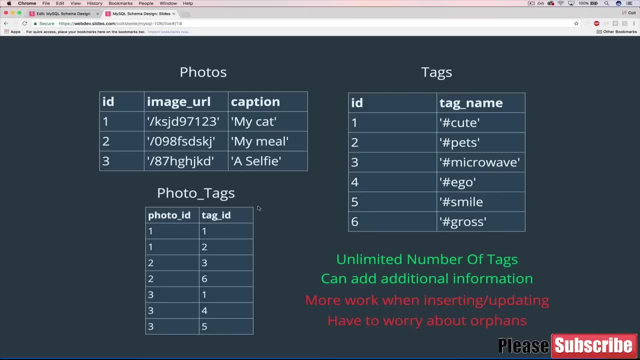 The advantage again, just like the previous one, there's an unlimited number of tags, and we can also add additional information, And so if I wanted to you know when a tag is created the first time over here, I could store the first time it was. 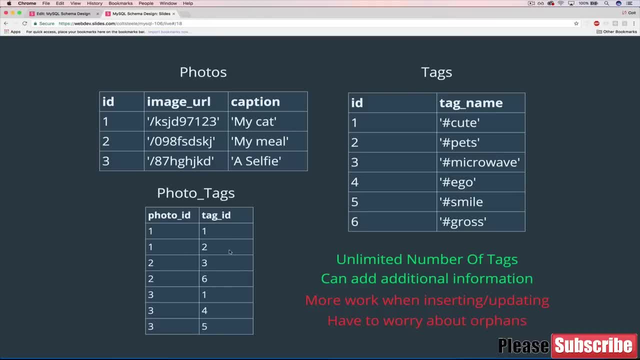 created and then over here every time it's subsequently used. I could store you know the time it was used or something, And so I'm sure there's some interesting data you could garner from that, or the location of where you know where in the world it was used, or something like. 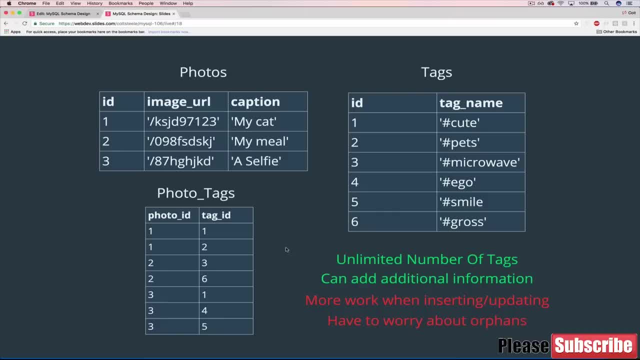 that the time of the day, I don't know day of the week, whatever, And we also have less duplication of the tags over here, But then there are a couple of problems and they really come down to just more work. So when we're inserting something, if it's the first time a hashtag has been, 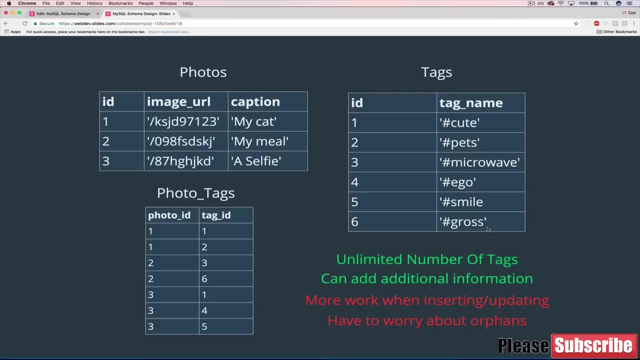 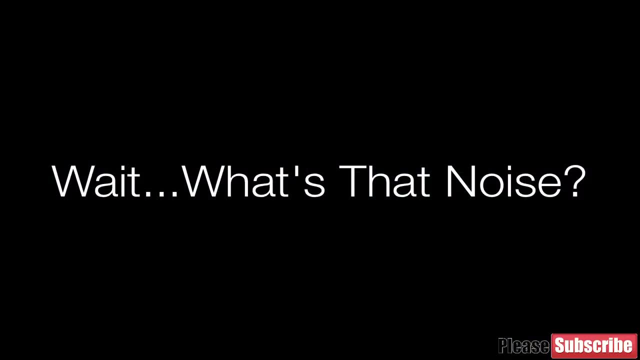 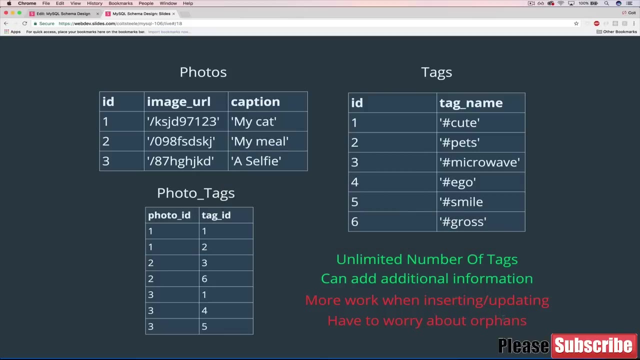 used and it's not in the database yet. we have to create it. and then we have to associate it with a photo using photo tags. And the same thing when we're updating, We have to What She just vomited anyway. And then we also have to worry about orphans. we should always all 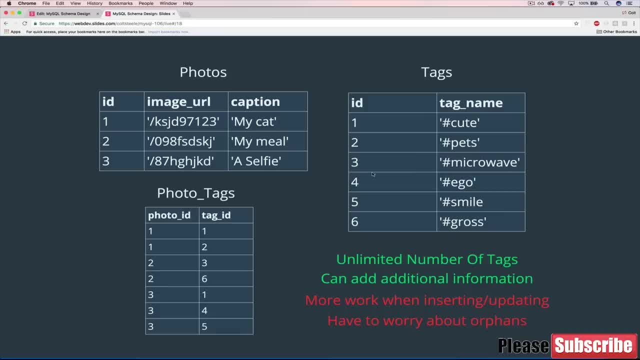 be worried about orphans, but in particular, when we're talking about these tables, when we're deleting something, right, if we delete a tag for some reason, which Instagram does you know if there's a problem? something is being misused or somehow being- you know, I don't know- controversial. 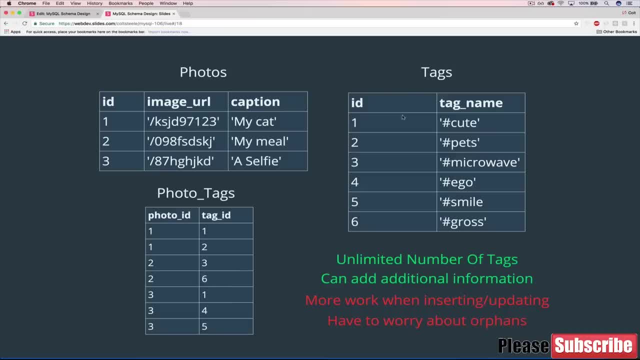 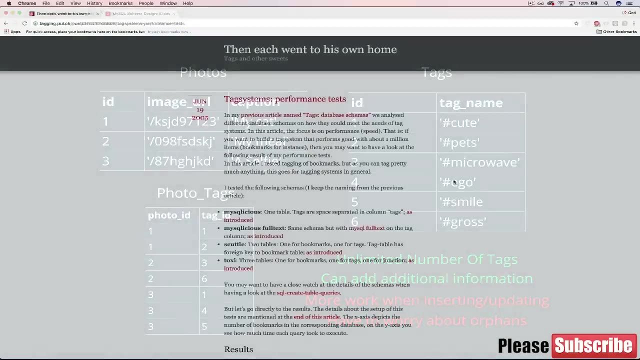 they can be removed, And so then we just have to make sure when we're removing it from here, we also need to remove it from all associated photo tags, So it can be a bit more complicated, but basically it comes down to that the cost of having this nicer structure is that it's just a little more work. 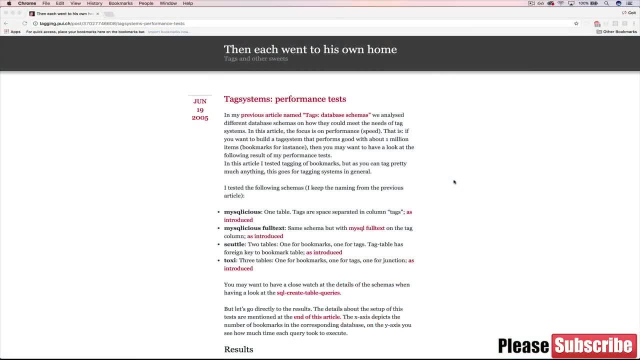 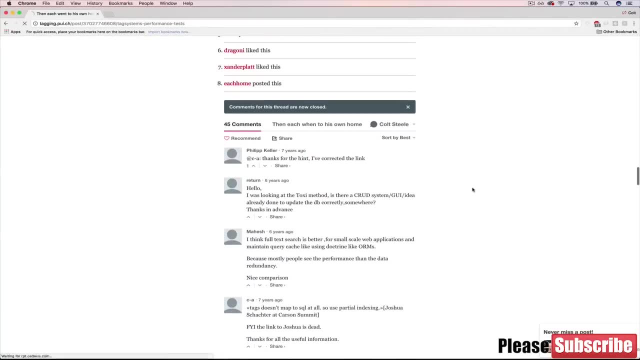 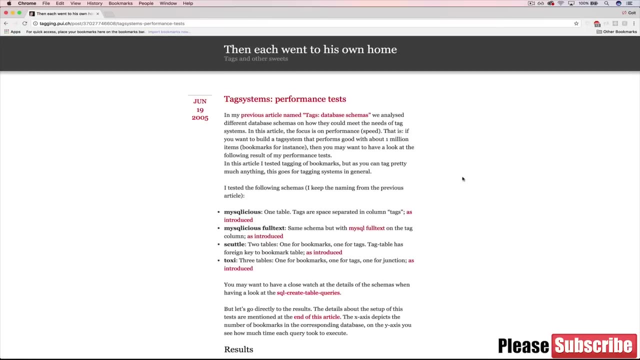 And just as an end note here, I did mention earlier that there is this great article online- this guy who does speed tests of different ways of doing tagging- and it's written up. include the link along with this video if you want to read it. I'll just spend 10 seconds talking. 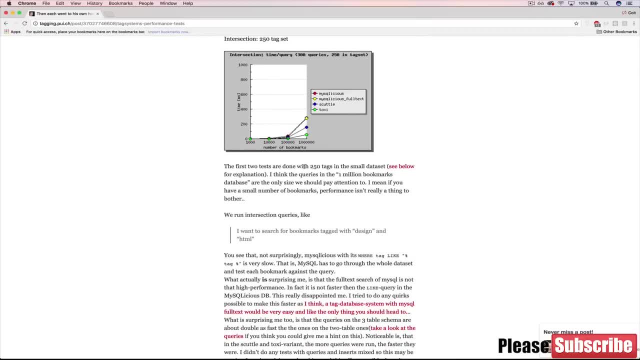 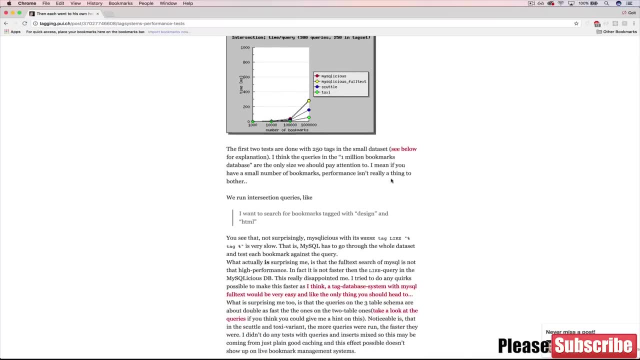 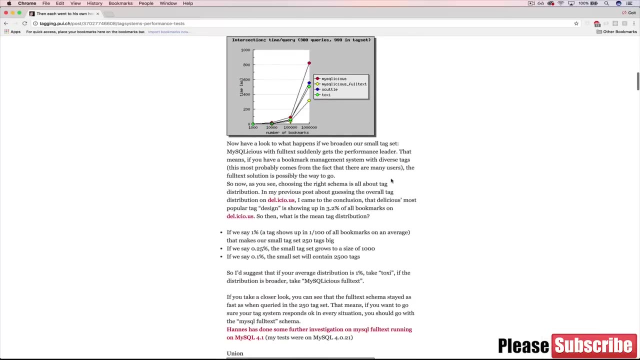 about it. but basically he does some tests here to show that, depending on one, the size of your data set. this example with a smaller data set, the second and third approaches I showed you with multiple tables are actually faster, but then as we get a larger data set with thousands of tags, it actually changes. 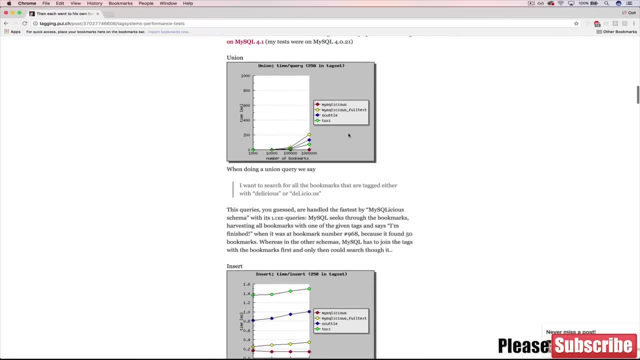 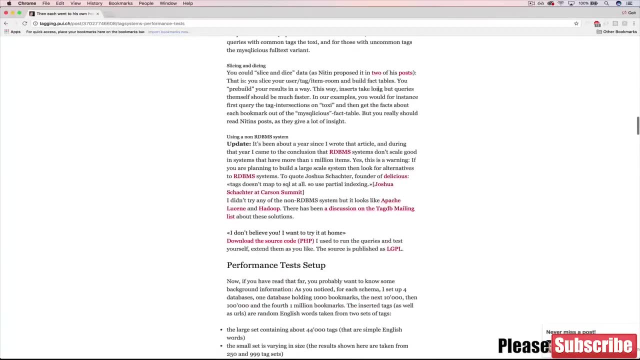 So it's just interesting to note that and to read. But also he talks about how much time it takes to insert compared to compared across the three different versions, And it's just an interesting article. But if you actually look at his conclusion section, which is probably what most of you 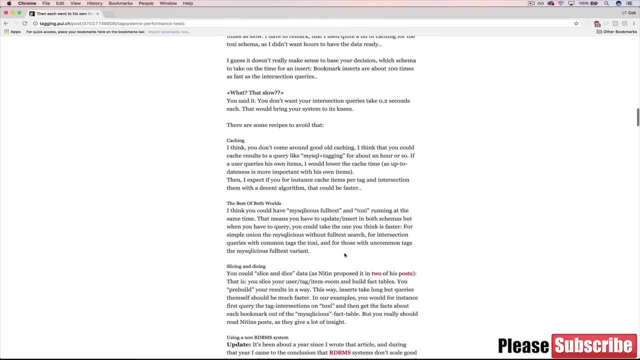 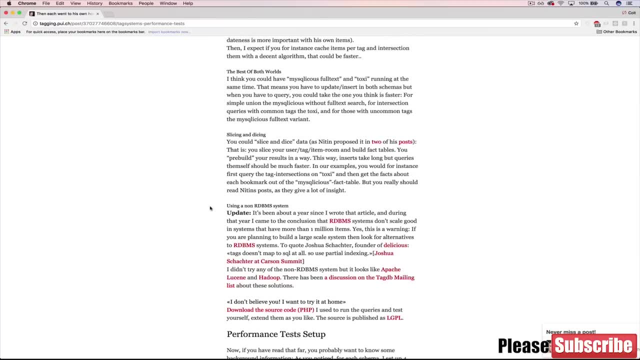 care about. where is that? Is that he actually thinks that it would be best to have, if you're working on a huge app, to have two versions- the- the first version I showed you and the third version I showed you- And basically they perform best at in different situations? 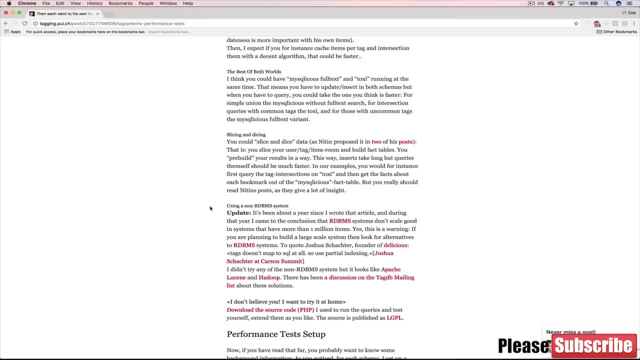 And this is getting into the woods a little bit, But basically the version that we're going to go with- the third one with three different tables- is faster If you're working with common tags- things that you know are used often- but if you're searching or you're trying to do joins with like rare, 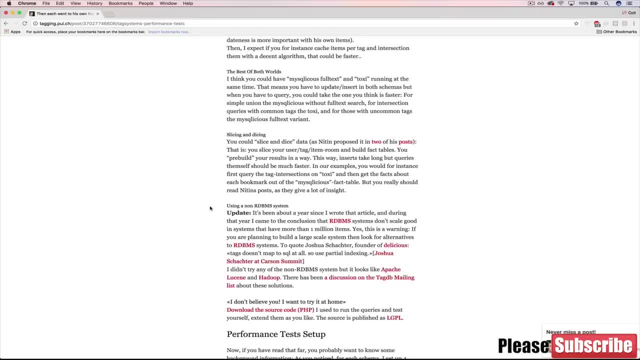 rare is the wrong word, but uncommon tags that just aren't used very often. then it's actually slower and it would be faster to do the first version. I showed you where you store them as text. So this guy is suggesting to use a combination of the two, which we're not going to get into. 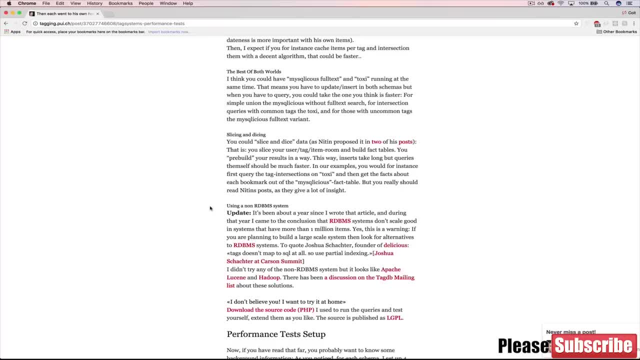 But just interesting to note that there isn't one best way and that it really comes down to your needs: What your app needs, the product needs dictate And, in all likelihood, as an app like Instagram grows, especially when it started out, to where it is now its schema. 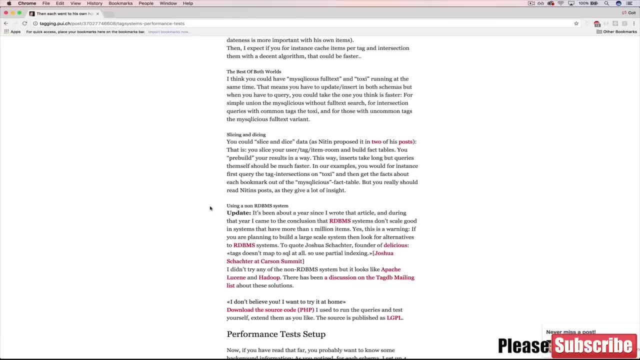 its database has undergone multiple big overhauls and changes, probably not just the schema itself but the database, whether it's going from something like MySQL to another type database or, a bigger change, going from a relational database like MySQL to a non-relational database. So it's really hard to say what's best. 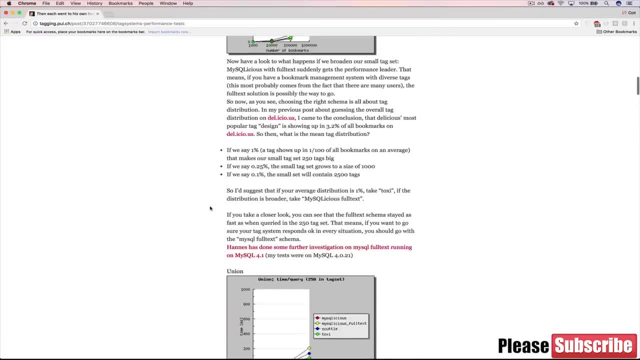 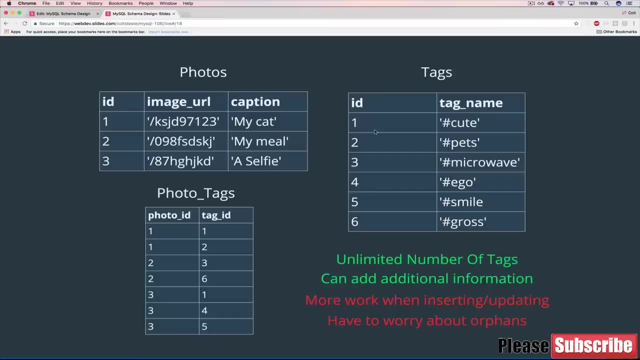 but it's interesting to take a look at somebody who's actually crunched the numbers And even after doing that, can't necessarily give a definitive answer, because the answer is: it depends. All right, So this will be a quick video where we just 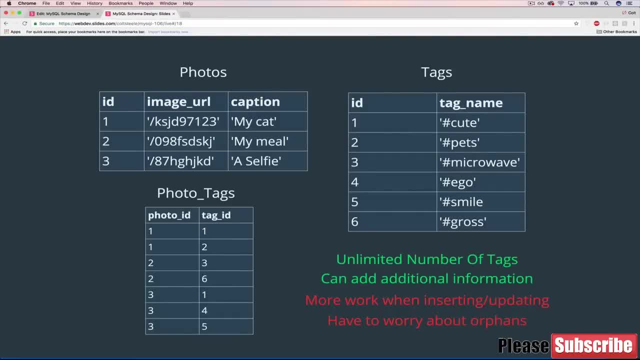 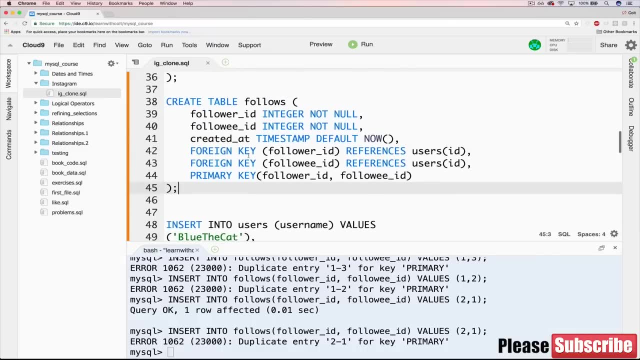 implement the two tables we need. They're both very simple. So tags is just an ID and a tag name. Photo tags is a photo ID and a tag ID. OK, so here I am in cloud nine and we'll start with our tags table. 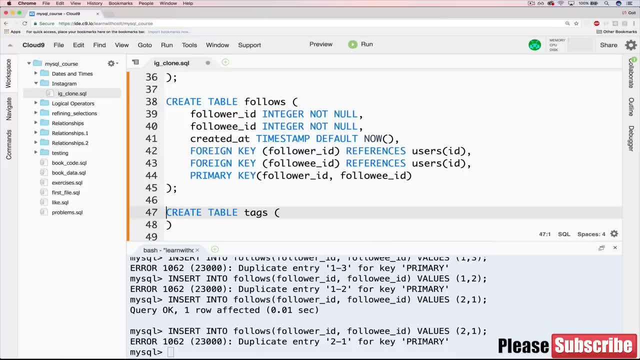 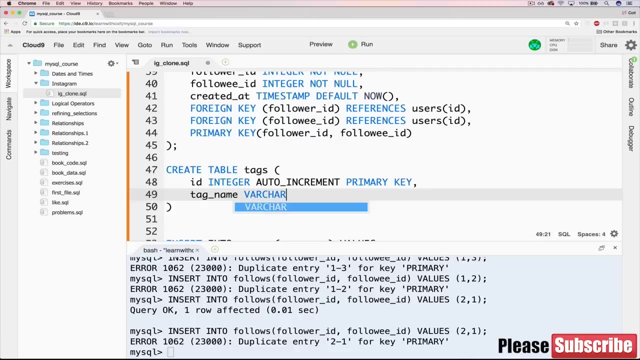 Create table tags and all we need is an ID which is an integer auto increment primary key, and then we'll also have our tag name, which is just a Varchar 255.. And we want to make it unique. We don't want to have- oh my gosh, I can spell unique. 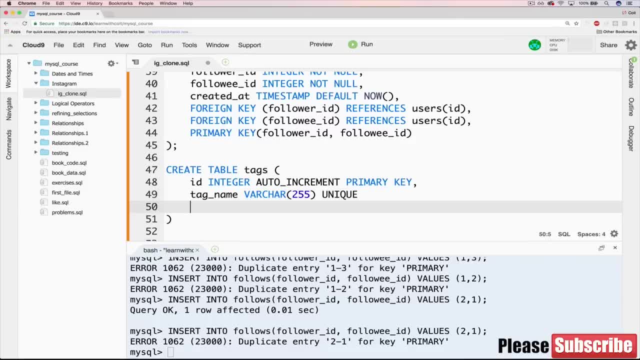 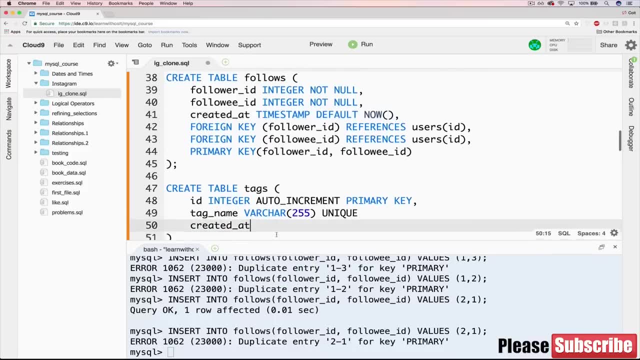 You don't have any duplicates in there, And then after that you know it would be nice to add a created at, like I said, so we could store the first time a tag was used or created And that's it. So that's our tags table. this table here. 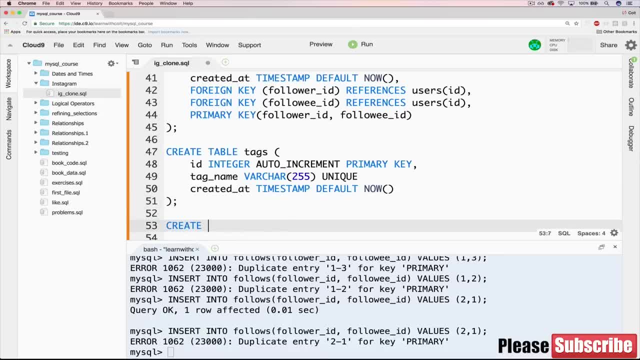 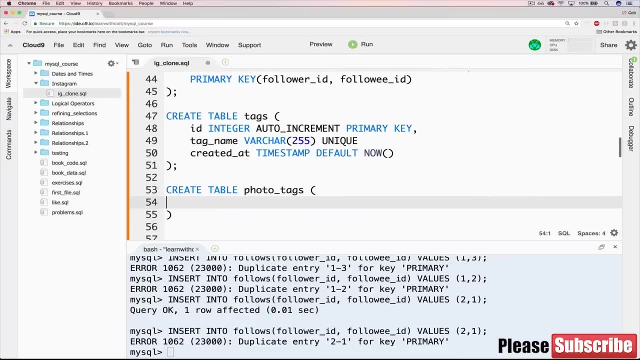 Now we've got to worry about photo tags, So we'll do our create table photo tags or taggings, which is also nice, I guess. Well, neither is nice, but also works. We don't need an ID. All that we need is a photo ID and then the tag. 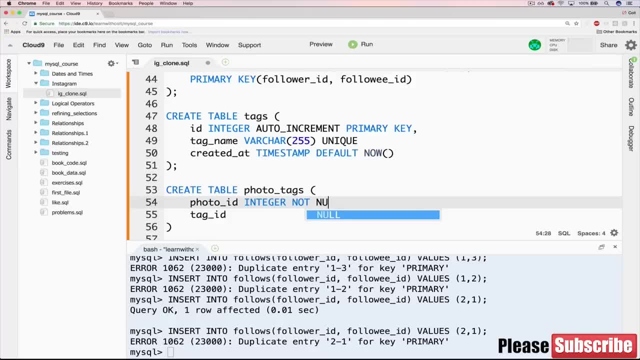 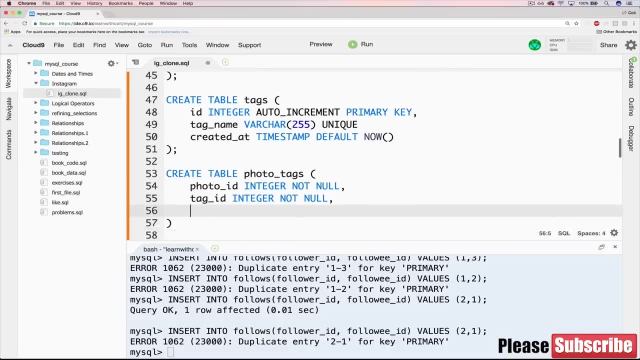 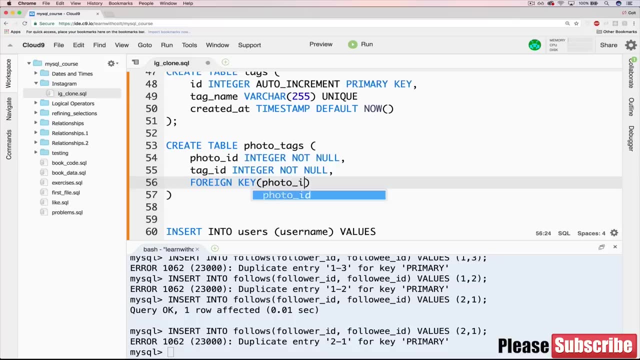 ID, And those are both going to be integer, not null. There we go, And then on top of that, we need to add our foreign key constraints. Foreign key: photo ID is referencing the photos table ID field. Duplicate that tag ID is referencing. 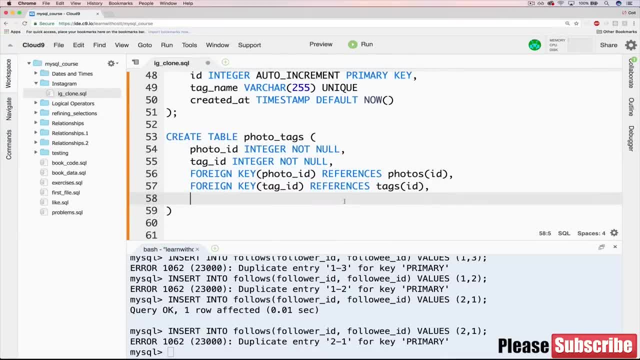 Tags- table ID field. We also want to make sure that a user can't tag the same photo with the same hashtag multiple times, And that's an easy fix. We just do our same primary key with two items: photo ID and tag ID. 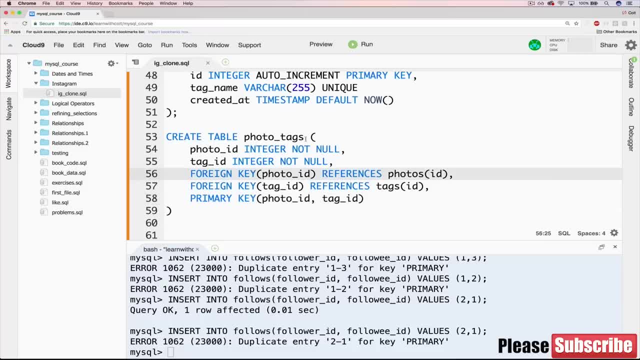 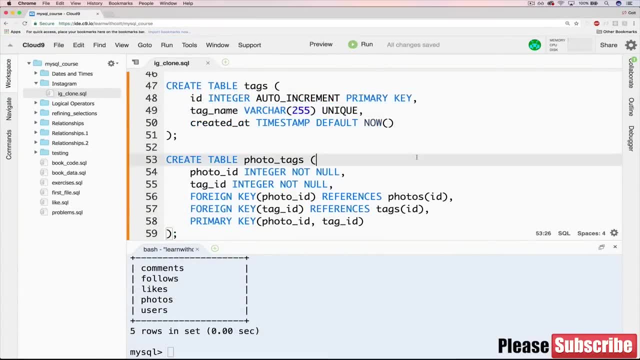 And that just ensures that we can't have multiple instances of the same photo tags. All right, Don't forget our semicolon. It looks like I'm missing this comma here. There we go. Now, if we try that And we look at our tables, There we go. 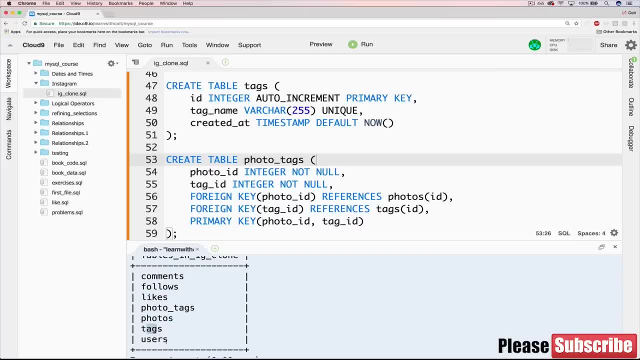 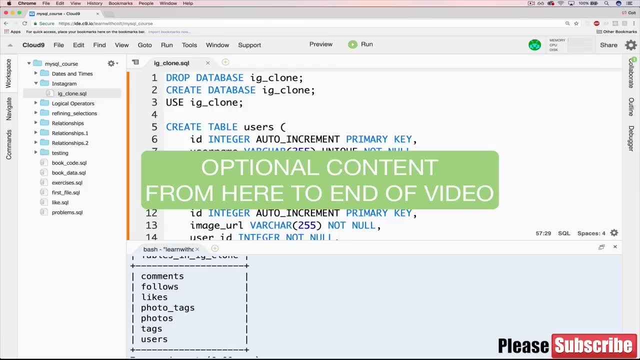 We've got comments, follows, likes, photo tags, photos tags and users, And that's it for our schema. We're done So in the next section. if you'd like to tap out now, move on to the next section. 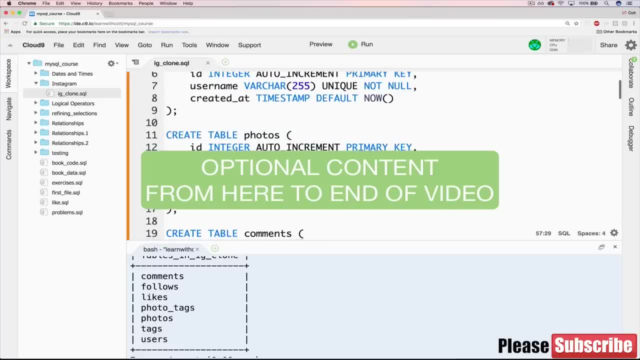 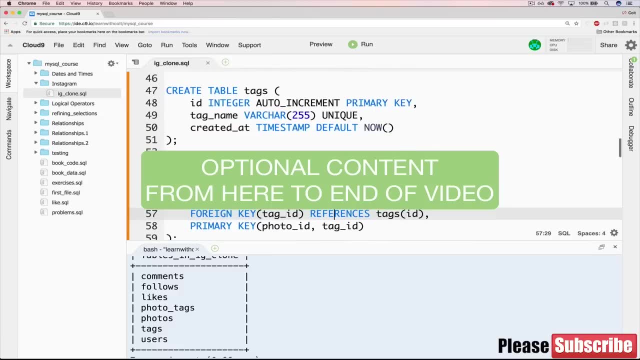 We're going to give you a massive file with a bunch of data that I created. took way too long to do that. We'll be able to do some exercises with and get some practice working with a bunch of tables. But if you do want, 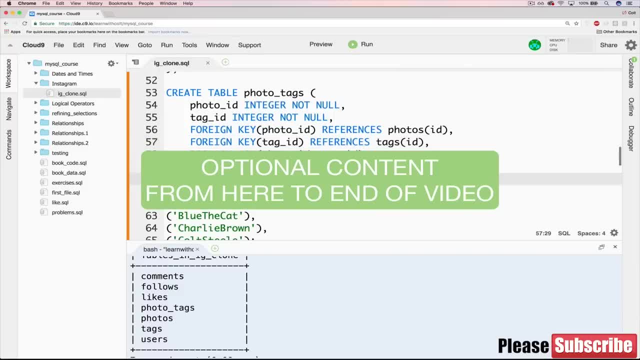 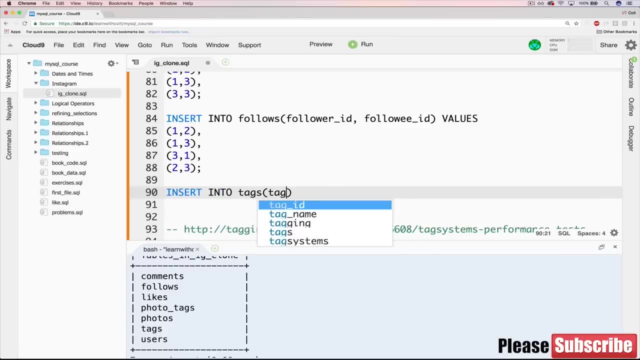 See me just insert a couple of tags and photo tags. I'm going to do that now. So, if you're still here, I'm going to do that. I'll start with inserting a couple of tags And all we have is tag name. 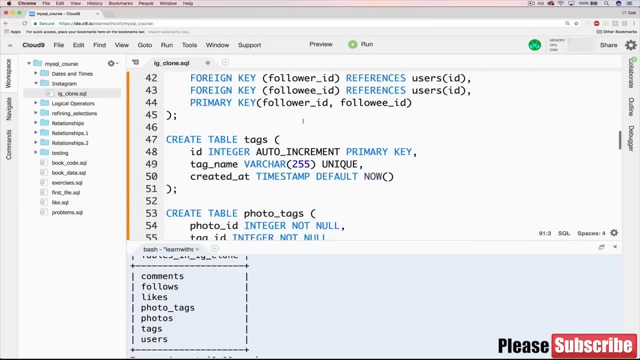 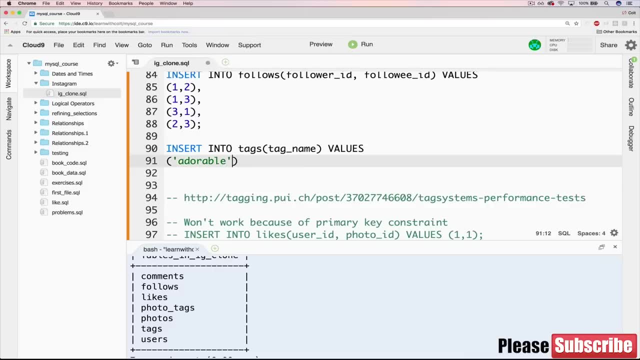 And just to verify that we go back up to our tags. it's just a tag name that we're inserting, so let's say I'm inserting the string, you know, adorable, And we get two more. Let's say cute, And one more would be, I don't know, sunrise. 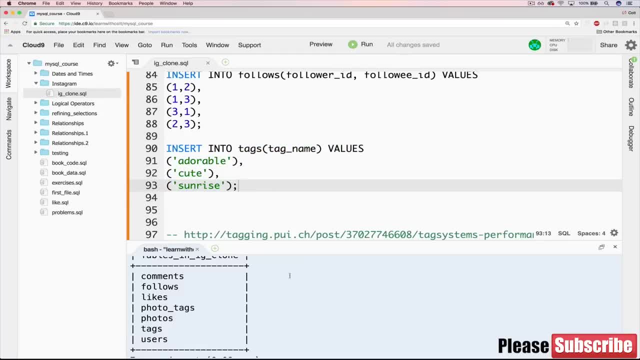 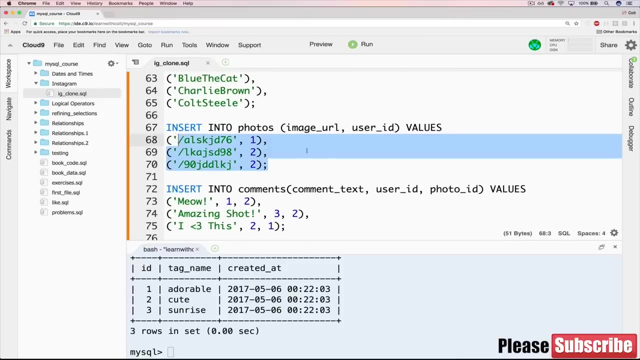 OK, so that will insert our tags. Can make sure that that works. Select star from tags. There we go. We've got our three tags. Now we associate them with photos, And so we've got three photos. You know it doesn't matter what they are, but they have an idea of one, two and three. 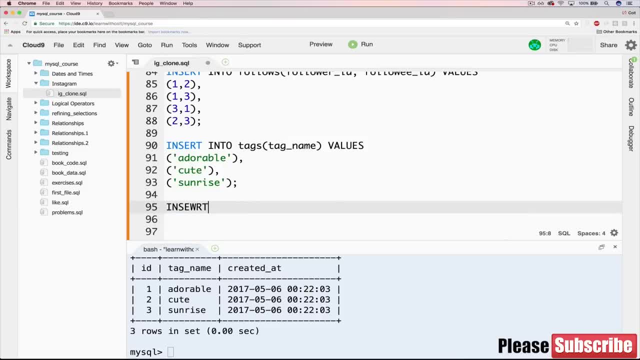 So if we want to do an insert Into- If I spell insert correctly- photo tags, We'll start by taking the photo ID and then the tag ID, OK values, and let's say the first photo is tagged with adorable. 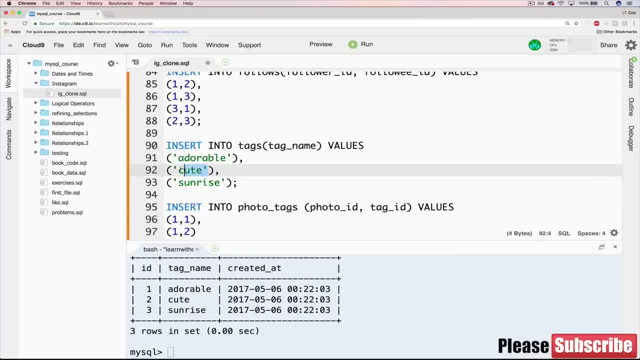 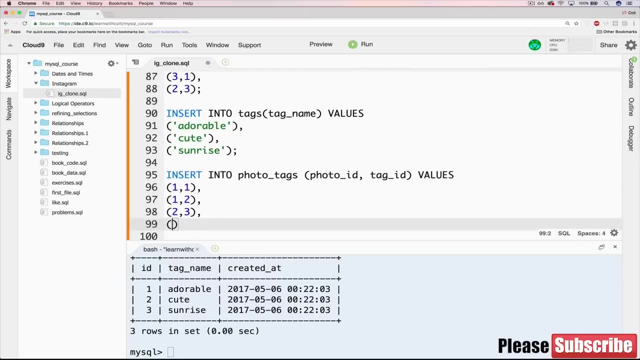 And the first photo is also tagged with cute because that has an idea of two. And then we'll say: the second photo is tagged with, I don't know, sunrise, And then the third photo is also tagged with cute, like that. OK, so we can rerun this. 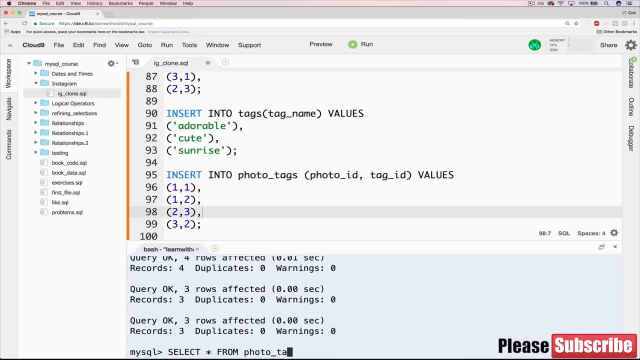 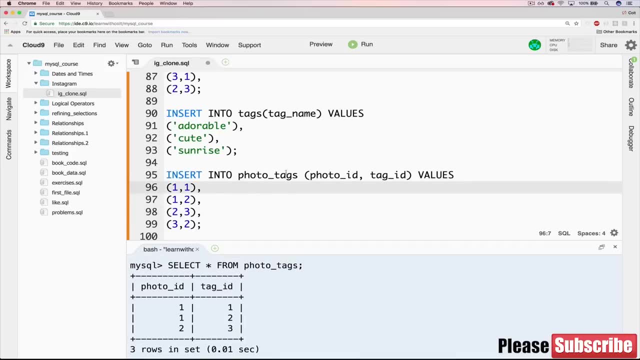 Let's do select star from photo tags. There we go, Looks good. And now the true test is: can we still insert something that shouldn't work like a duplicate? we already have, you know one comma one, So insert into photo tag. 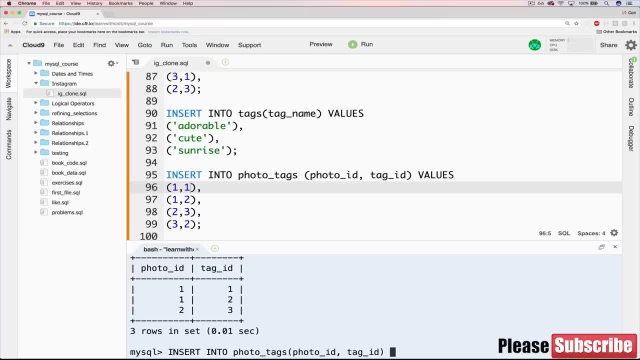 Tags: photo ID, comma tag ID values: one comma one And we get duplicate entry. So that's good, Works perfectly. But as you can see, you know the other order works fine. Two comma three or three comma two are not the same thing at all. 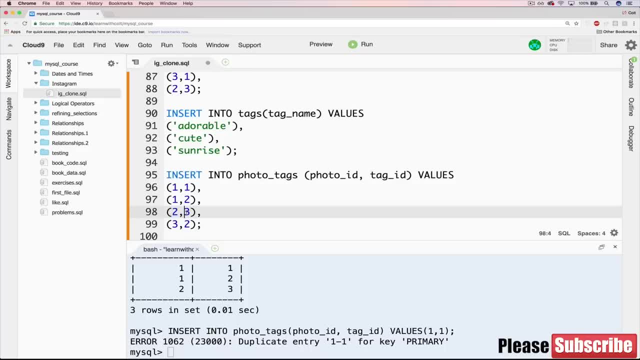 This is saying the second tag. or this is saying the second photo should have the third tag. That's this is saying third photo should have the second tag. Quite a mouthful, All right, So we're done here. Next up, We're going to play around with data. 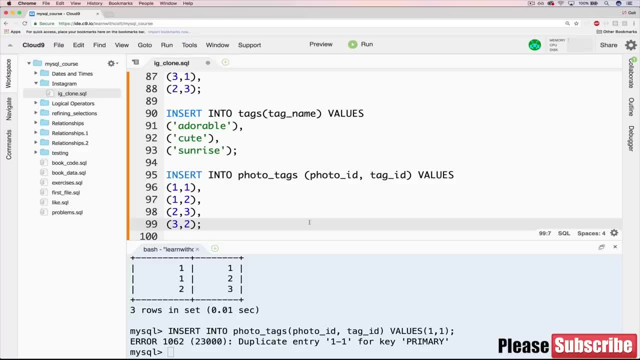 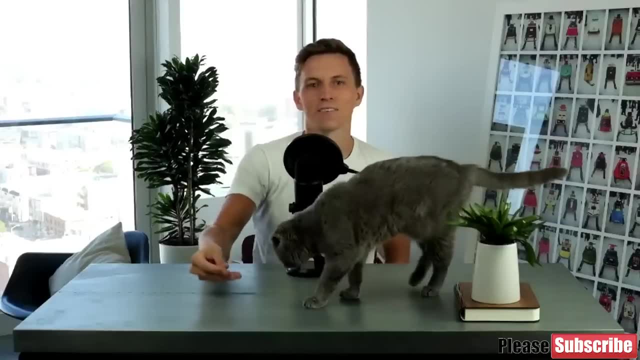 Like I said, I'm going to give you a giant file. Hopefully it's fun, And if it's not, well, we're basically at the end of the course, So just hang in there. Hey, welcome to the next section here. 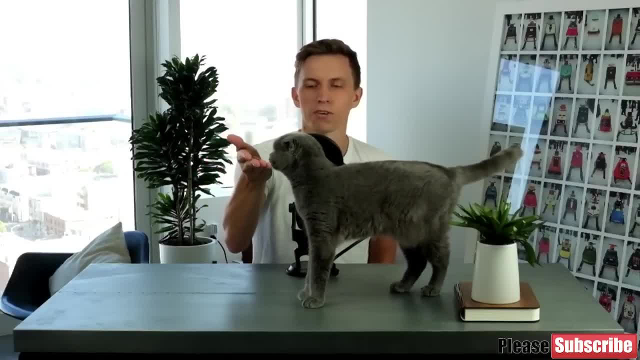 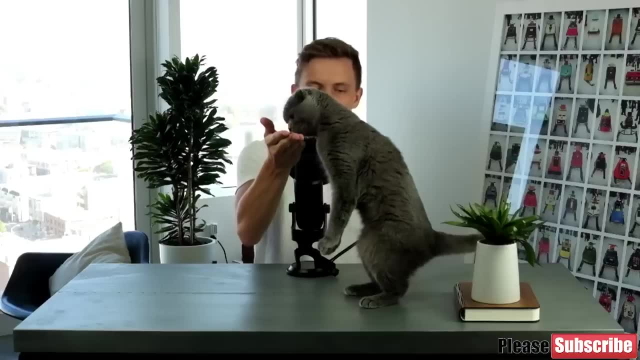 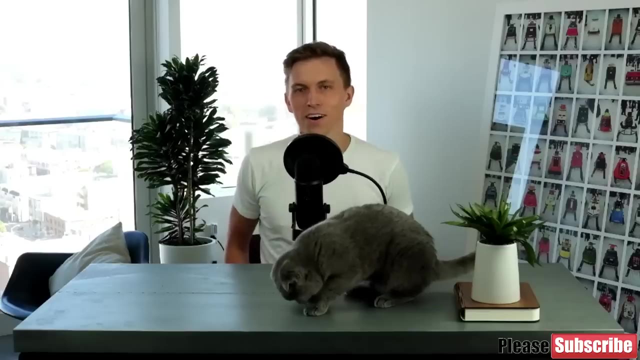 This one. we're continuing with our Instagram data and see if Blue will do her trick again. Blue, Can you get it? Oh, who is my adorable little kitty? You can stand up like a human. She's come so far. You have come so far. 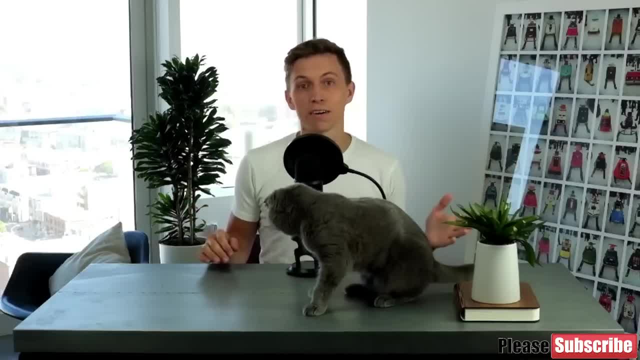 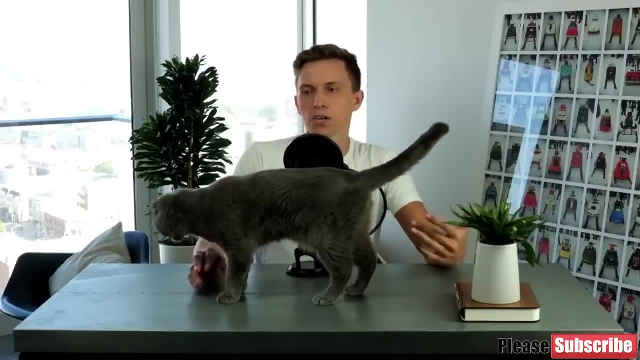 Yeah, So we're working with Instagram data. We set up the schema. Now all we have left is to do stuff with it. So the way this section works is, rather than me giving you a bunch of tables showing you, here's the result I want. 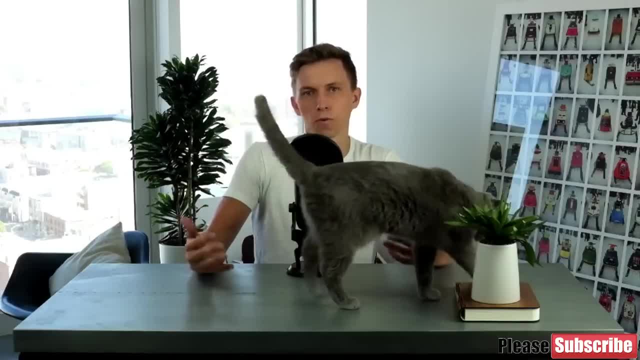 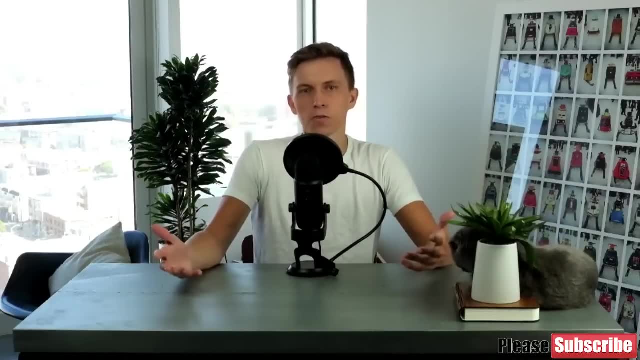 We're going to do it a bit differently. I'm going to ask you more of a real world question like: hey, we're doing a sweepstakes, or how about we're doing a campaign, email campaign to email all of our inactive users and send them. 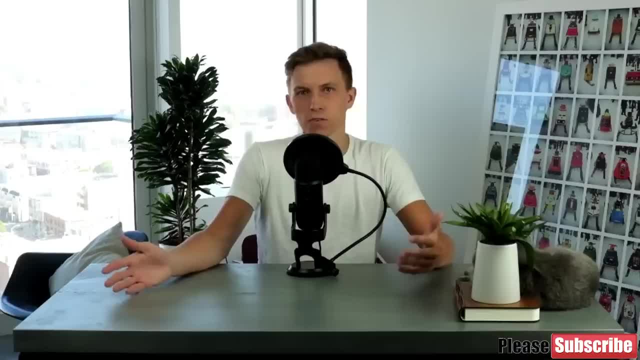 a reminder that they should post. So we need you to get all the inactive users email addresses, So something like that, where it's kind of in real world terms, not in the terms of a database like select all users, where blah, blah, blah. 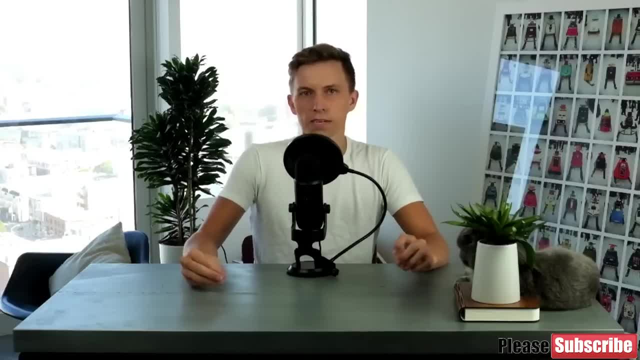 But you'll have to translate it, So we'll do things like that, or we'll do things like: hey, we have a brand who's really pressuring us to figure out what hashtags are the most useful or what are generate generating the most likes, and they want to know what three hashtags. 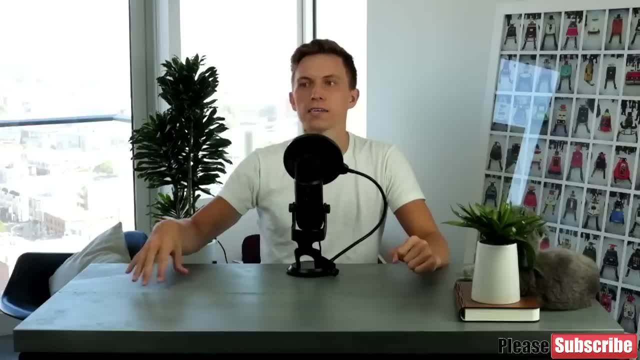 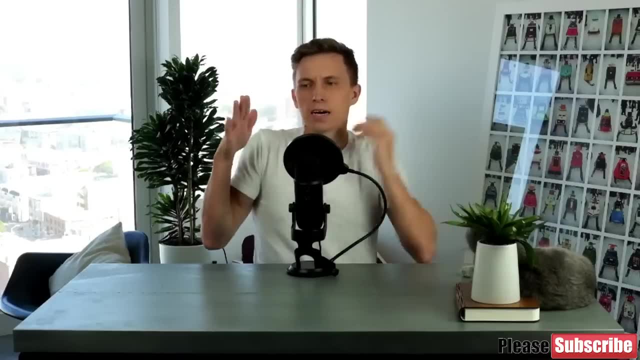 they should use. So then you'll have to go Write the query to find that answer. What are the best hashtags? How do you know? So hopefully that's exciting, Trying to make it kind of a nice ramp off to the real world, just for the data. 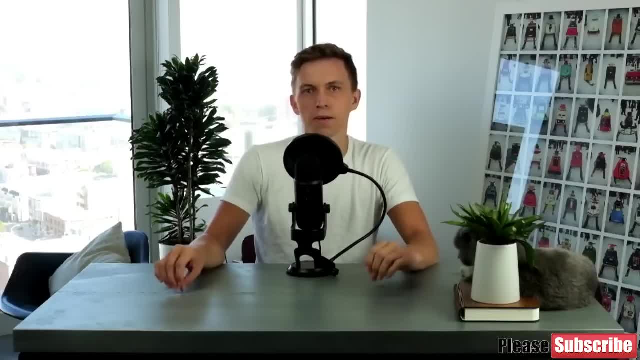 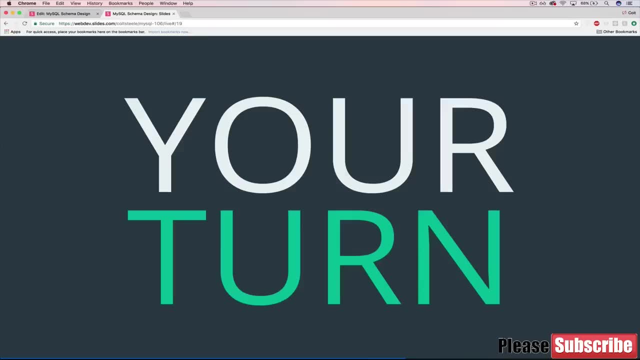 section And then after this, like I said, we have the Web app portion of the course. OK, so lots of exercises, all exercises and solutions in this section. Goodbye, All right, Welcome to the next section. So what we're going to do here is basically take the schema design we came. 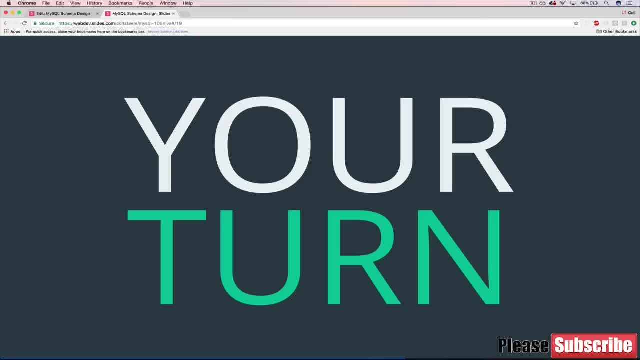 up with in the last section for a roughly Instagram ish application with photos and users and comments and tags and follows and all of that. We're going to take that schema and implement it And I'm going to give you a bunch of data to put in your database. 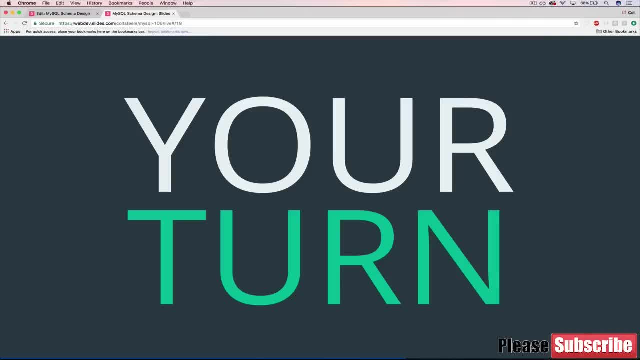 like a couple thousand of things to enter. I wrote a giant file and what we'll do is put that in there, So we all have the same starting place, And then we're going to pretend that we're the company and we're trying to figure out certain things. 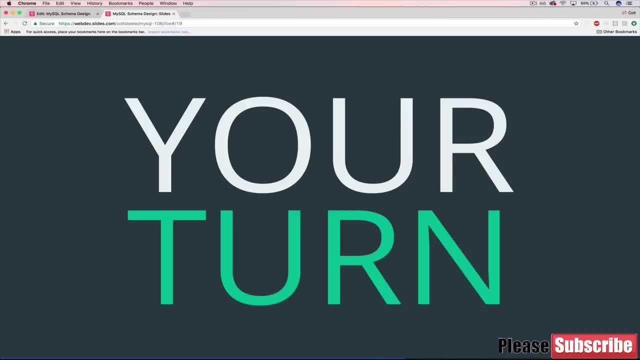 Like: do we have too many bots on our application? Are there user accounts that are inactive? Are there user accounts that have never posted a photo? Maybe we could send them an email campaign, you know, encouraging them to post a photo, or what hashtags tend to be most successful, that kind of stuff. 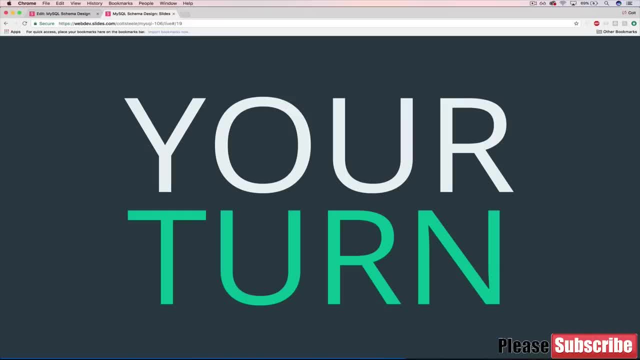 So all of this section, every video, will be asking a question, which is basically a nice way of saying. it will be an exercise, But we're now posing it rather than me just giving you a table, which is what we've been doing. where you know it's a table. 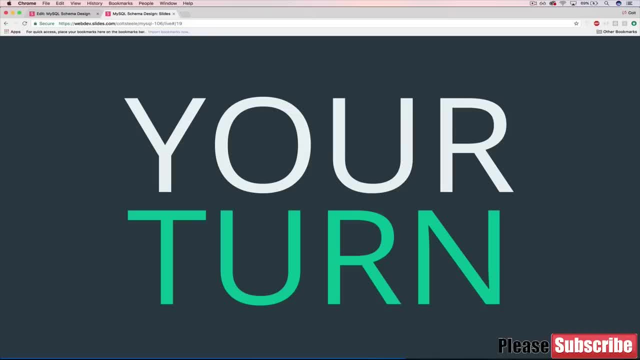 And I just ask you to recreate this. I'm now going to pose the question as if we work at a fictional company and we're trying to find something out. For example, it might be something like we're running a new ad campaign and we 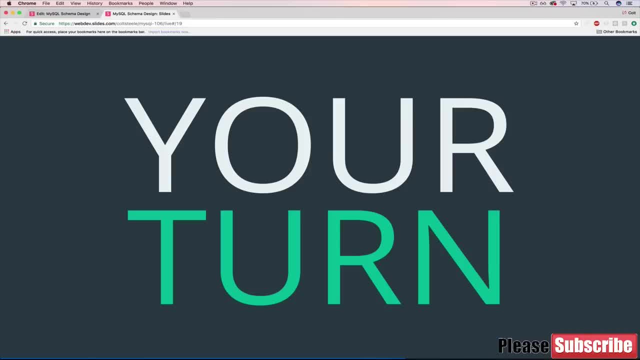 need to figure out which five hashtags get the most likes, something like that. So that's how this will work. Every video in the section will be a question And, rather than having all of the solutions at the end, making a giant video that takes like half an hour to go through, I'm just going to break them up. 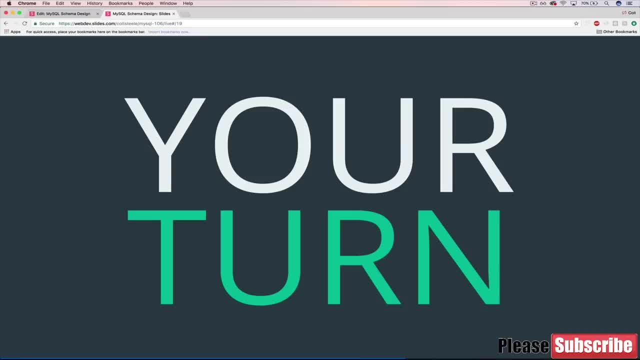 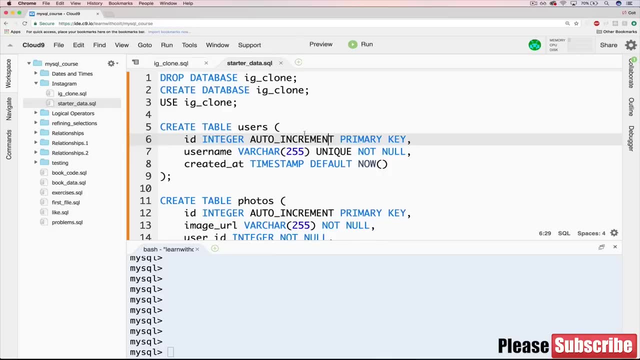 So every video will have the question at the beginning and then a following solution, But the first thing we need to do is insert all of our data. So included in this section is this file here, StarterDatasql, And there's two components. 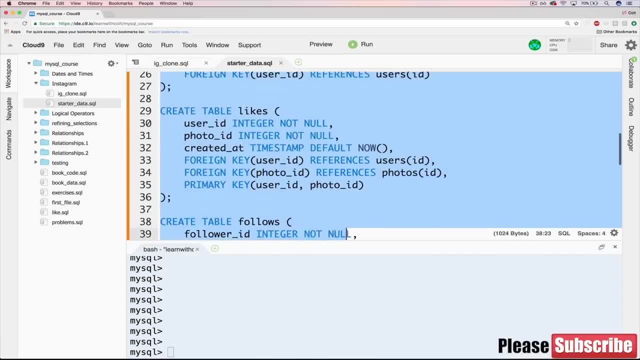 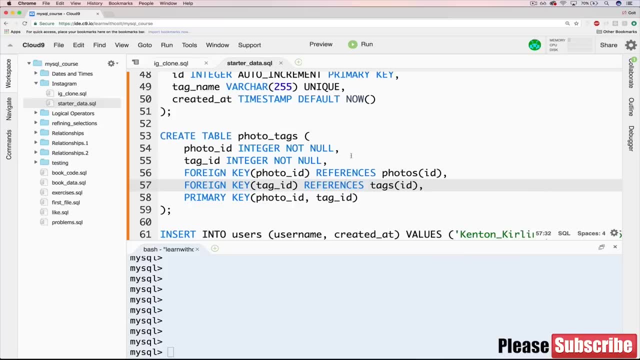 The first one is setting up our schema, and there's nothing new here. We talked about all of this in the last section, But if you were following along and doing it yourself, you may have named something slightly differently, Like, instead of photo tags. you may have called it. 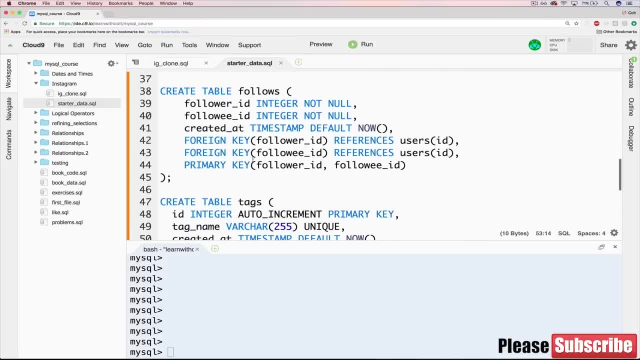 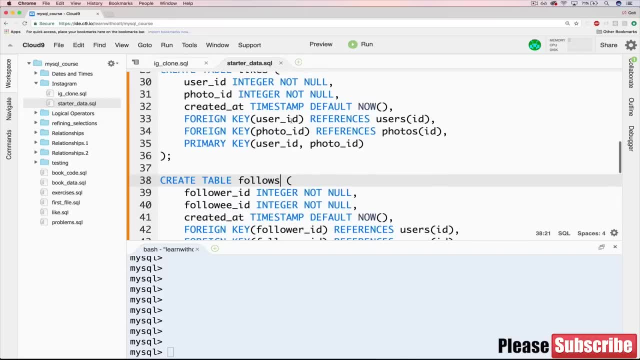 taggings or instead of- you know, I don't know- instead of following and follower and follows. maybe you called it following or relationship or something. So in order to give you this data here to insert, I needed to make sure that we all 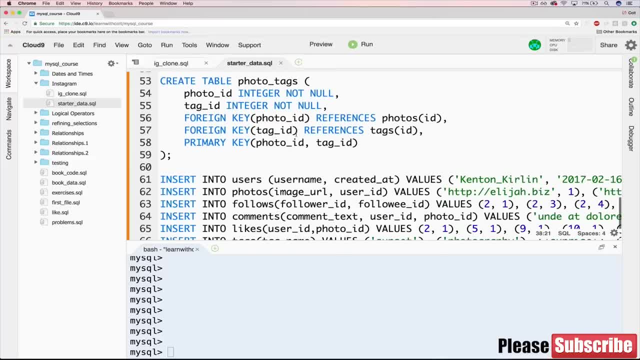 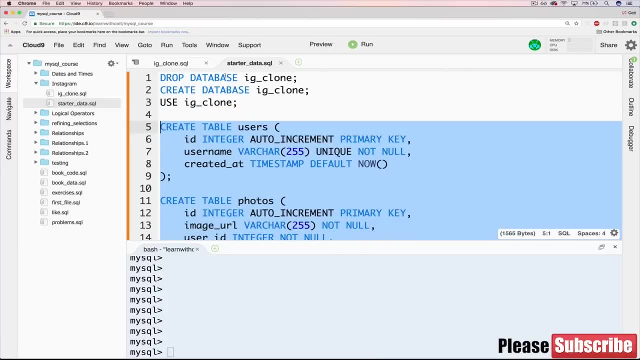 have the same schema, even if just one thing is named differently. It's a problem. So the first part of this is just a bunch of create tables- all the tables we discussed, as well as dropping the existing Instagram clone database, creating a new database and then using it if you wanted to. 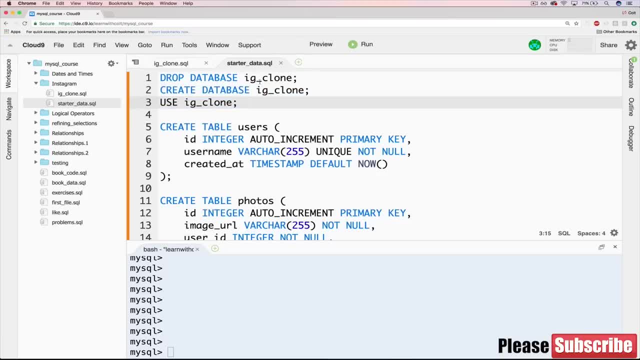 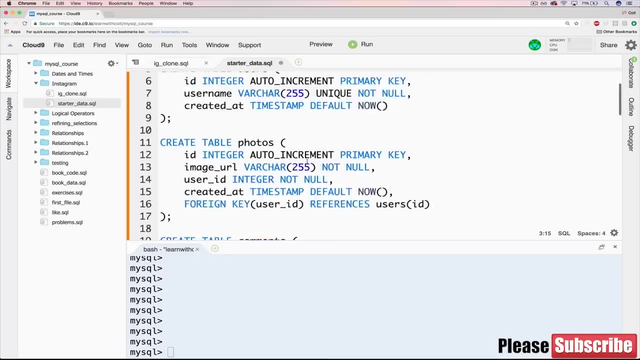 If you want to keep your current Instagram clone database, if you've been working with that, just give this a different name, whatever you want. Well, but you need to do it to all three of these. OK, so we set up the schema. 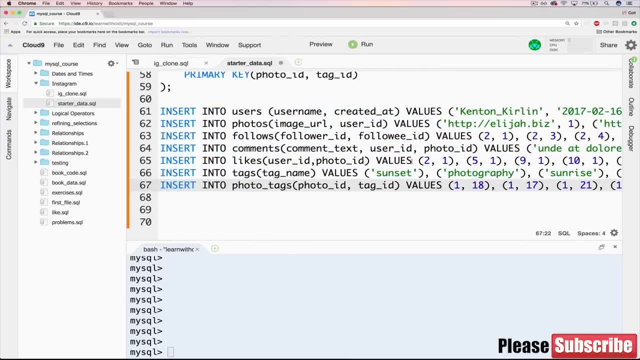 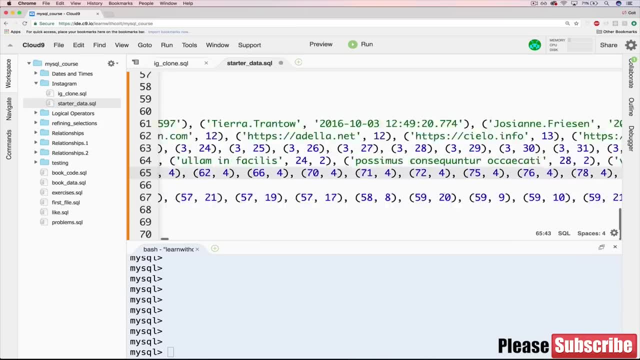 But then the fun part, which is all these insert statements, And it doesn't look that impressive when you look at it in cloud nine because it doesn't wrap them onto new lines. And if I start scrolling you'll see I'm scrolling really fast. 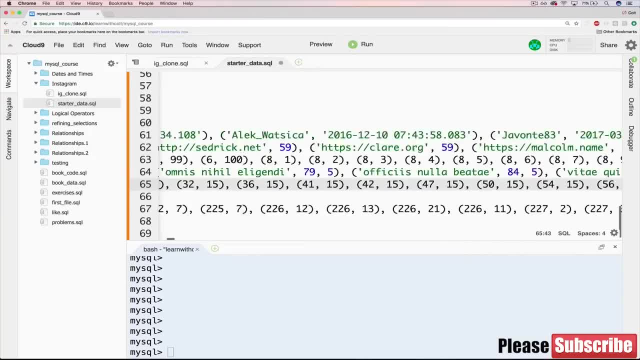 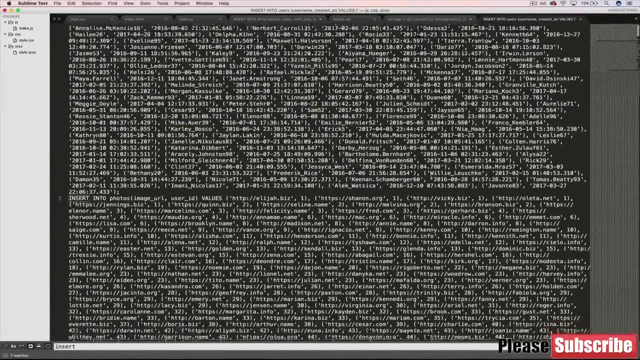 But look down here in the progress bar I've barely made a dent, And this is not a great way to visualize the data. So instead, here I am in sublime text and here's the file that I generated. It's the same exact file. 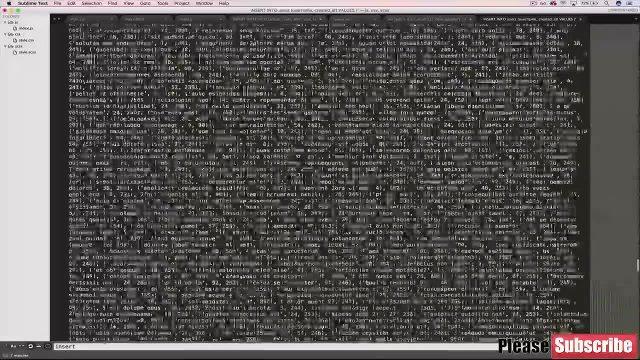 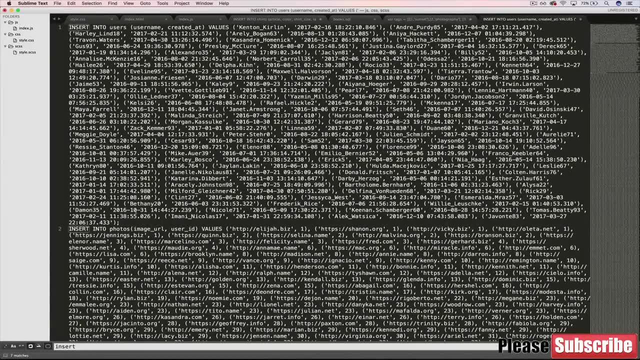 It's just displayed all here. rather than having to scroll across, I have to scroll down. So you know we won't do any sort of grand tour of the data, but I will say this: I spent a lot of time trying to figure out how I wanted this to work. 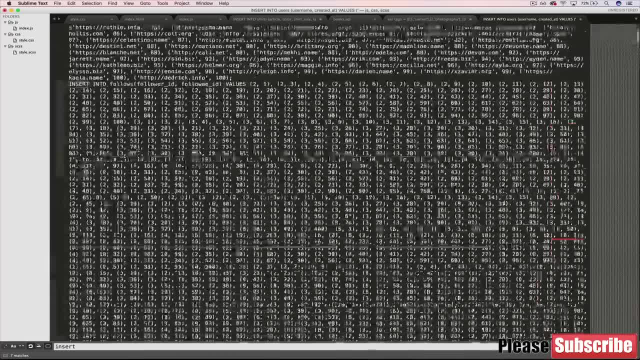 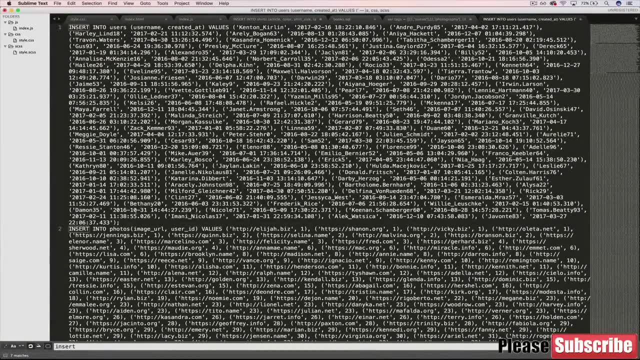 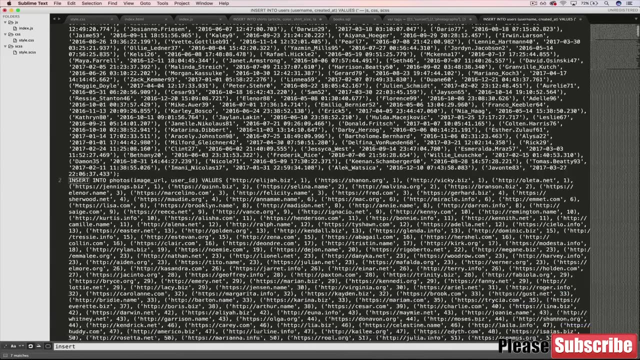 Obviously, I didn't type this myself. I would have taken like days probably. Instead, I wrote some code which still took probably an entire day and a half to get this how I wanted, because I didn't want just randomized data if I just wanted to insert a bunch of random users and posts. 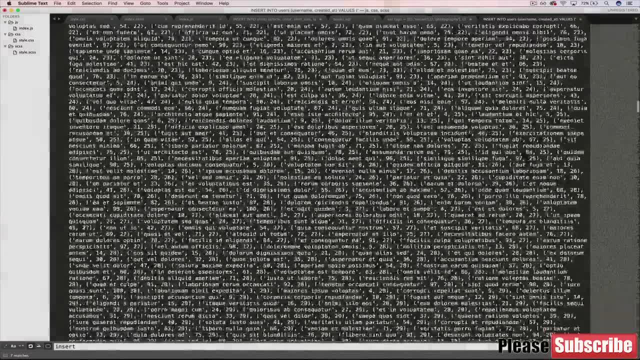 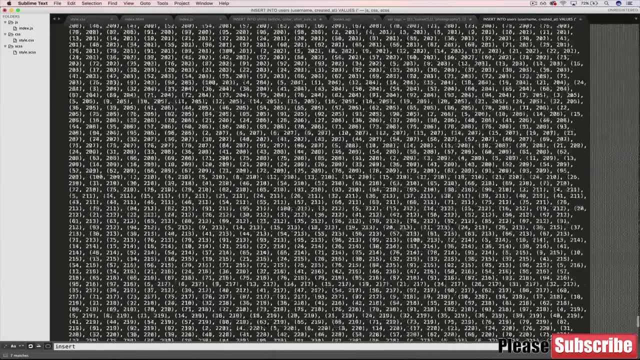 and comments that have no meaning to it. I could have done that pretty quickly, But instead I tried to design this so that there is certain personas to our, to our users. So some users post a lot, So they have a lot of comments, a lot of posts. 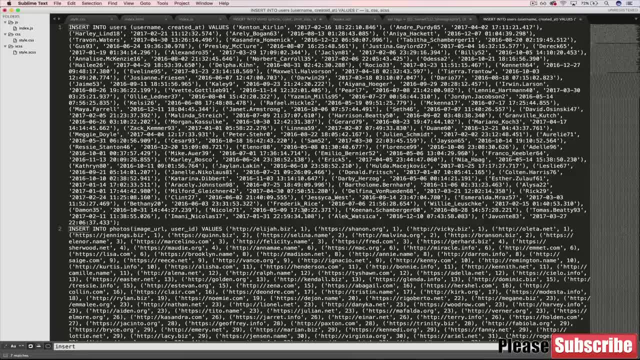 Some users are lurkers, meaning that they don't really do anything except look at people, maybe like certain things at best, but they don't comment and they don't post. Then we have things like bots, which on Instagram, are a real problem. 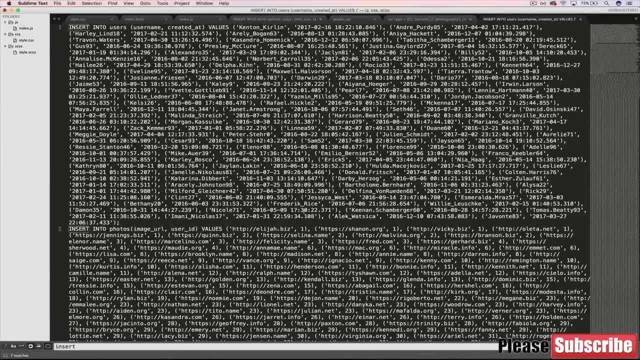 where bots are accounts that exist basically to go out and like a bunch of things, comments on things, usually the same exact comment, but they don't post things. And then we also have, like celebrity accounts who have very few people that they actually follow, but they have tons of followers. 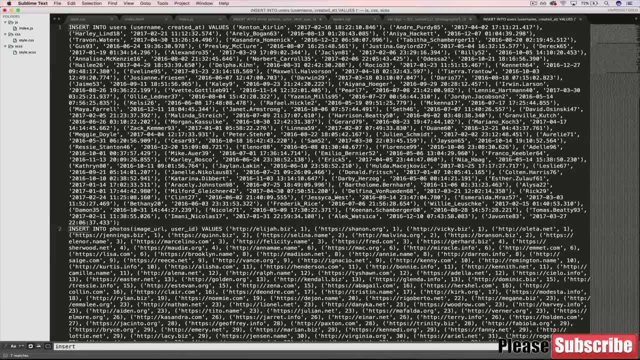 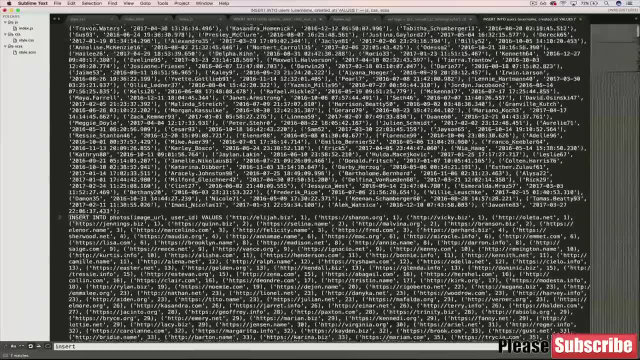 and they're not very active with commenting or liking, but they're very active with posting. So then we've got things like hashtags, and I didn't want to just do a bunch of random hashtags. I tried to actually come up with combinations of hashtags that. 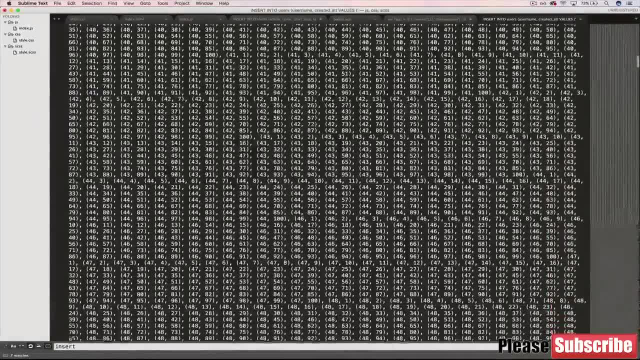 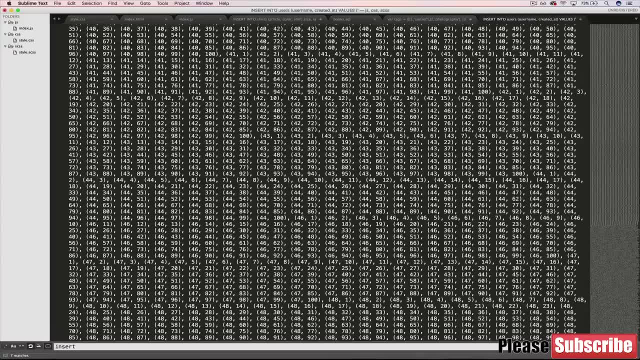 would be common. so you know, things like smile and style and fashion might be together often, but then we might also have smile and party or concert. those might go together or we might have, you know, landscape and sunrise and sunset and beach. 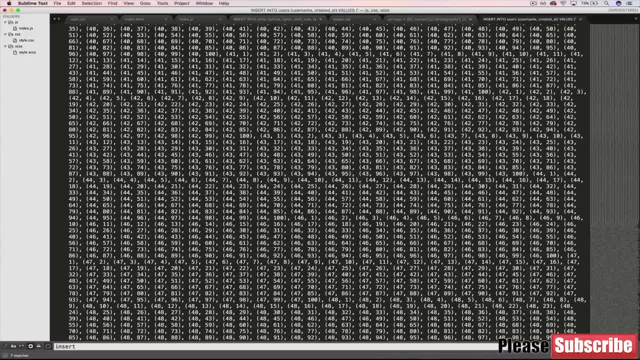 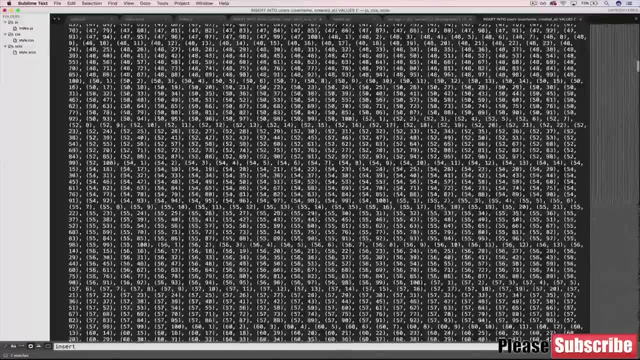 could be a combination for a beach photo at sunset, But then we could also have beach with party or beach with beauty or something like that. So that's just kind of scratching the surface, But I tried to design a lot of that in there so that we had somewhat realistic data. 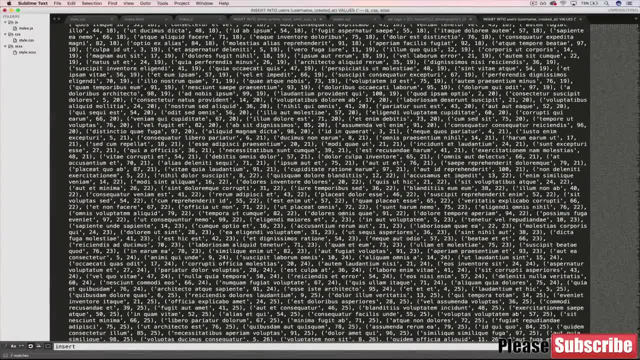 With that said, things like comments. the text of a comment is just random lorem ipsum text, So there's nothing there. you know that's going to be meaningful about the comment itself. What's more meaningful is the relationship between the comment and who posted it, and 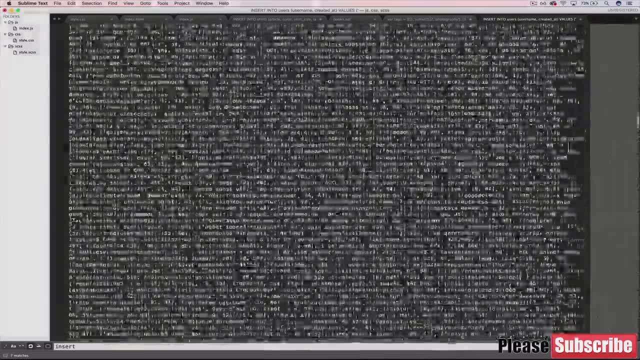 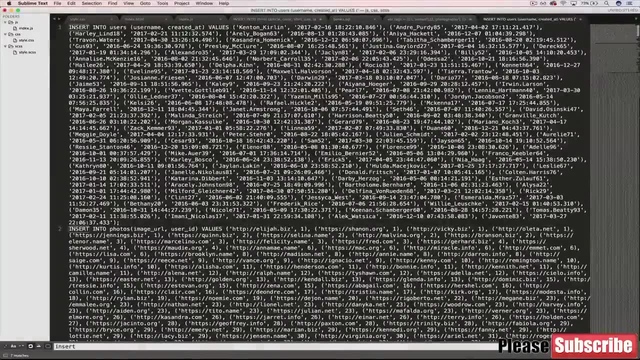 if they have a lot of comments or they don't have many comments and that sort of thing. OK, so that's enough of that. So, even with all the effort that I've put in here, there's still only, you know, 100 or so, or exactly 100 users, about 250 something. photos: 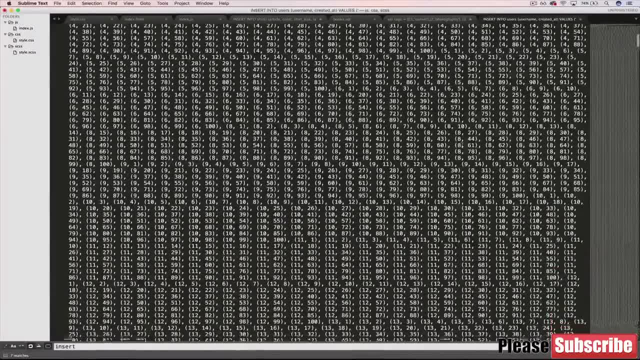 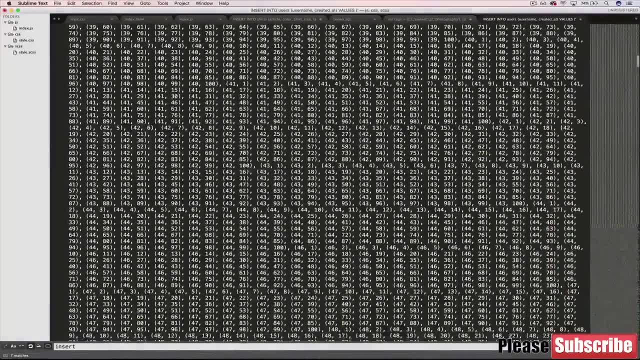 But then when we start talking about likes, there's thousands and comments. There's tons and following or follows, whatever we called it. There's tons and tags. There's only maybe 20 hashtags, But then when you apply them to all of those photos- 200 photos. 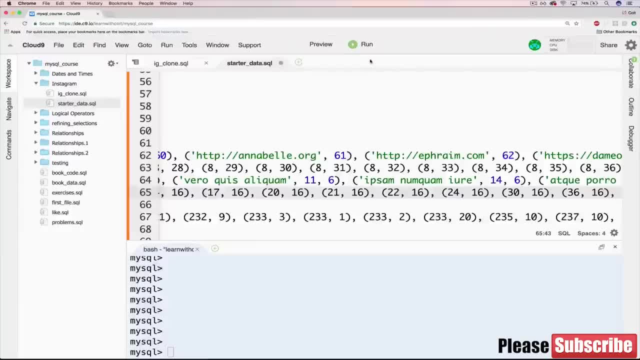 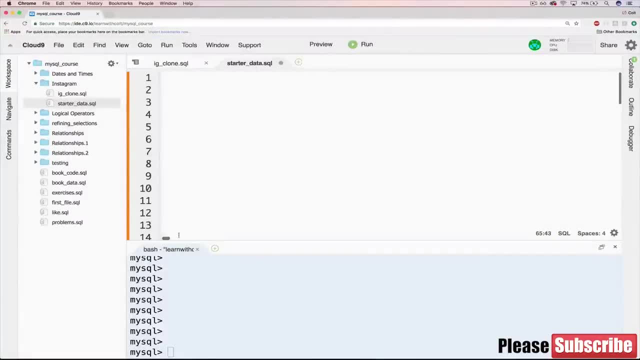 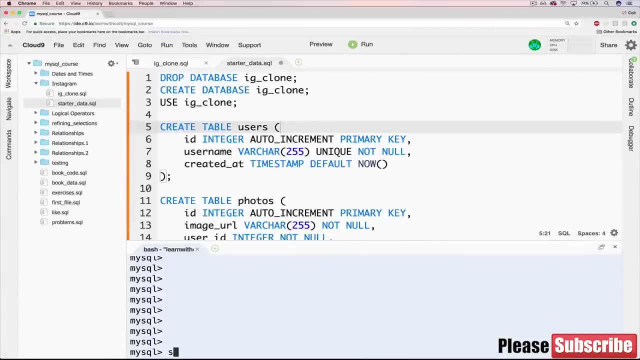 we get thousands to your thousands of instances. So all you have to do is get that into a file and then execute that file. Let me scroll back over, It'll take too long. Oh boy, Almost there, Here we go. So execute this file, and I'll just do that now with source. 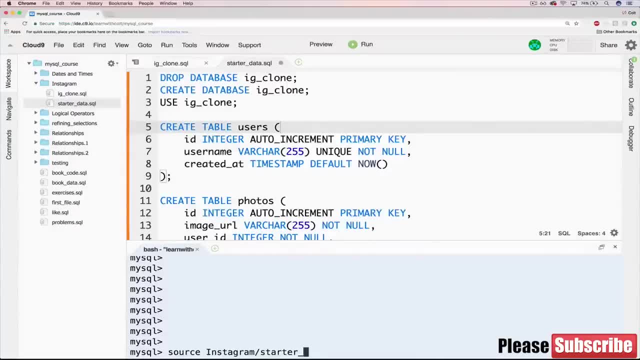 Instagram slash starter data, and that should just be the path that corresponds to wherever that file is and whatever you named it. OK, So it takes a little bit compared to what we've seen so far. so if you take a look, we've got a bunch of tables being created- seven I think- and then a bunch of things. 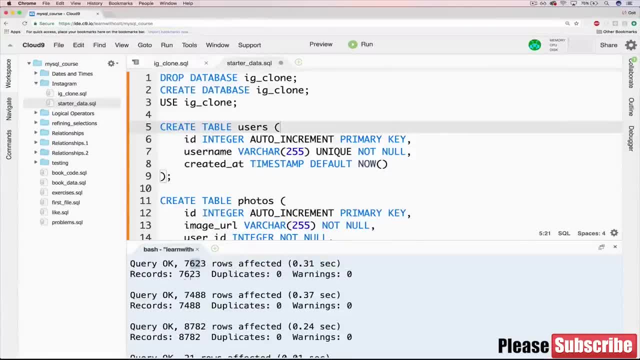 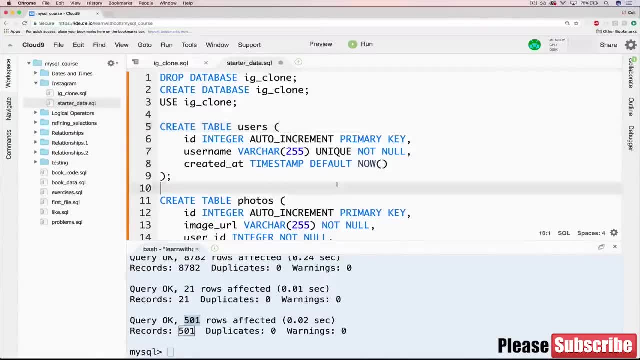 being inserted: one hundred two hundred fifty seven, seven thousand six hundred and twenty three, seven thousand four hundred eighty eight, eight thousand seven hundred eighty two, Twenty one and then five hundred one. So this is still a very small data set compared to- I mean, tiny. 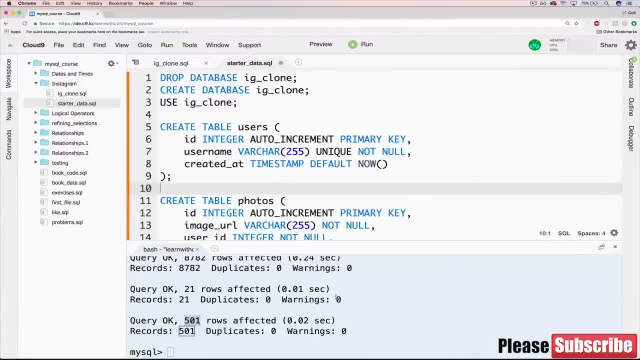 minuscule compared to Instagram. this is maybe like a minute of Instagram activity or probably less than that- a couple of seconds as far as the number of photos and stuff, but it's still an order of magnitude greater than what we've been working with. 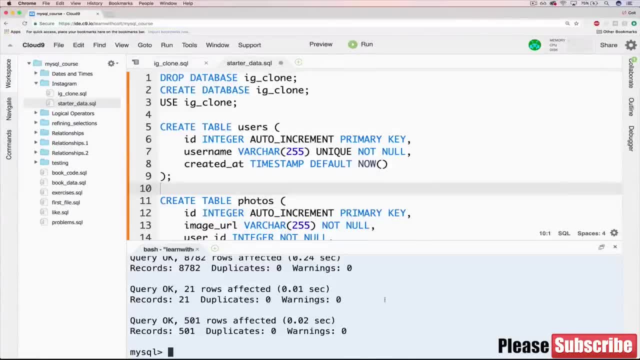 One other thing that I'll show you is that we haven't really seen giant amounts of data like this, And if you try and do, let's do a select star from likes, which I think we have a lot of You actually, if you, if you start to scroll through it. 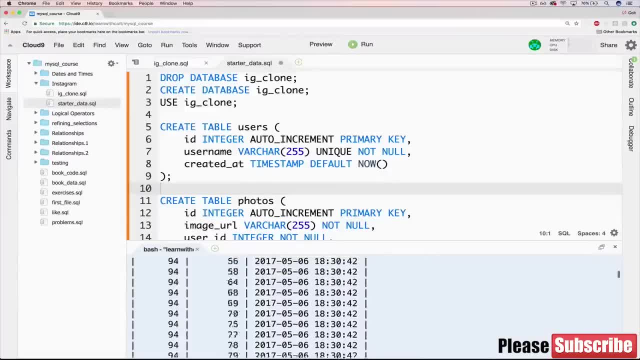 you'll see that we're not going to be able to see all of them. There is a number that we, that the terminal or that the CLI will print out for us, and then it just gives up or decides not to display all of them. That doesn't mean they're not there. 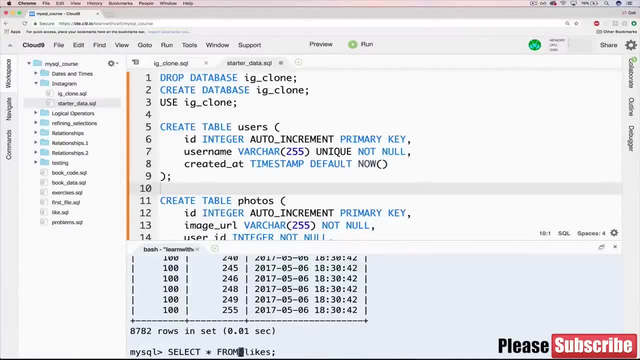 So if you did a count, for example Count star from likes, we get eight thousand, And if you join them with another table, it will join all of them. It just won't display everything. So for some reason you needed to display every single like. it would be better not. 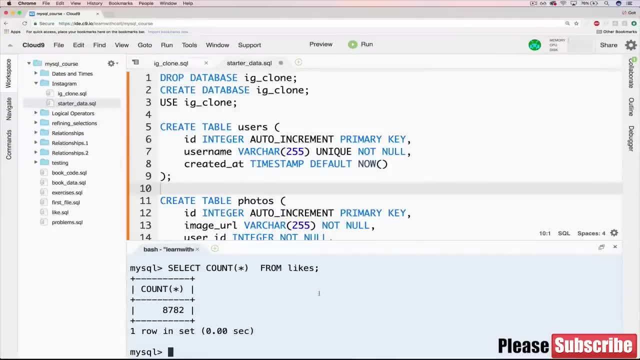 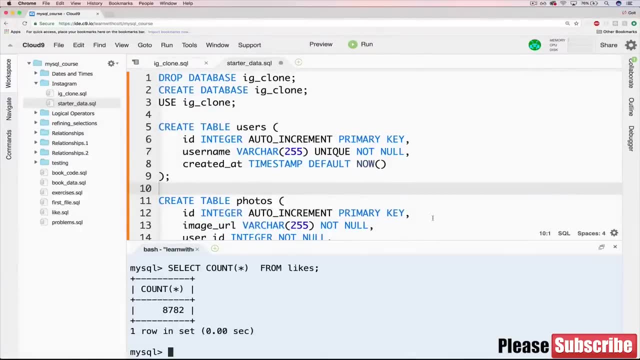 to do it using the CLI, but to do it from another file or some code somewhere. Anyways, so that's it. We've got the data set up. If you'd like play around with it, explore it a bit and then we'll start with our fun challenges in the next video. 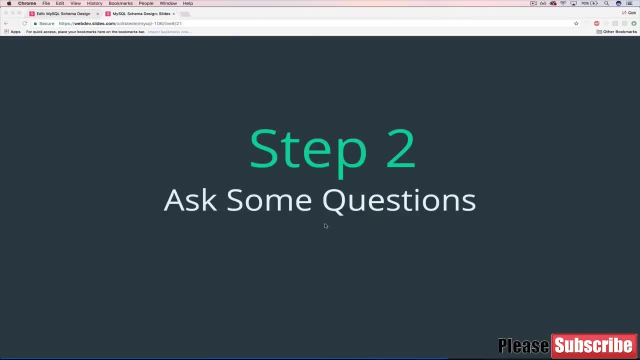 All right, So we have this data in our Instagram clone database. Now we're going to ask some questions, And the reason I'm phrasing it that way- asking some questions- is because that's usually what you're actually doing If you work with SQL SQL, some SQL database or any database. 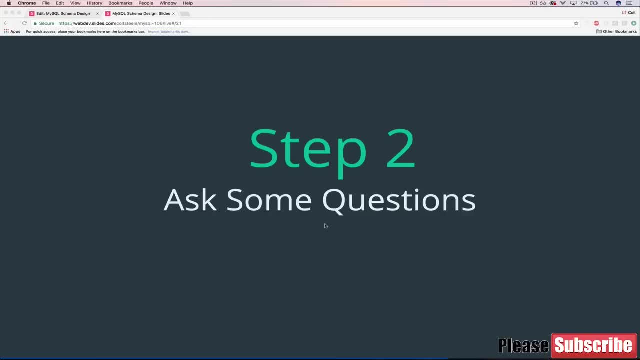 really, even if it's like a MongoDB or CouchDB, Postgres, MySQL, any database out there, and you have a bunch of data in there. Yeah, sometimes a lot of the time you're just sticking stuff in there, But when you're actually working with the data and writing, 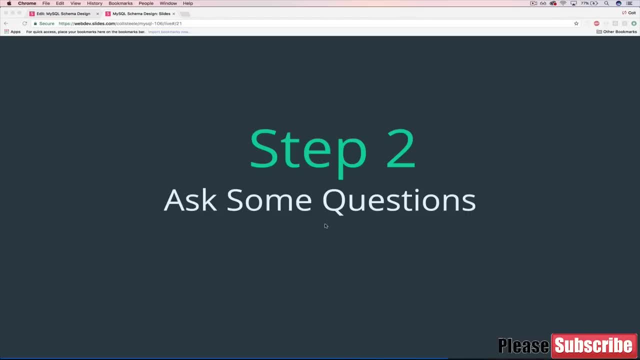 queries. a lot of what you're doing is asking questions where you have a motivation. You're trying to figure something out, whether it's for an ad campaign or a postmortem after a campaign. I know I'm coming back to ads a lot. 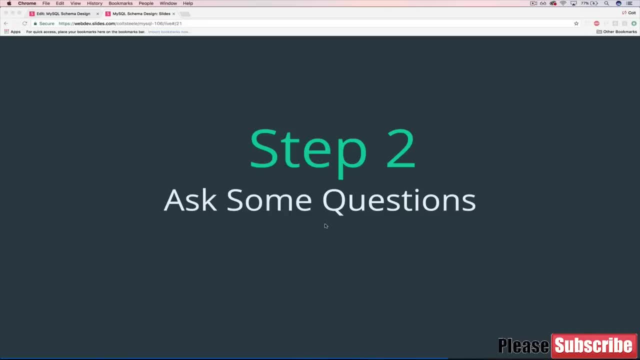 It might just be sales. like you could be a woodworker, You make furniture and you want to figure out how much you sold last year, because you're compiling your tax returns or something and you need to figure out the total volume you sold. Those are the questions you're asking. 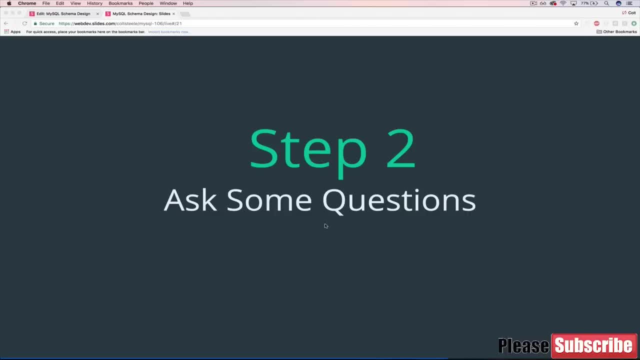 So you think in terms of English or whatever language you speak. you think in terms of questions in a non SQL language like how many X did I sell last year? And then you have to translate that to a sum or a select something from something. 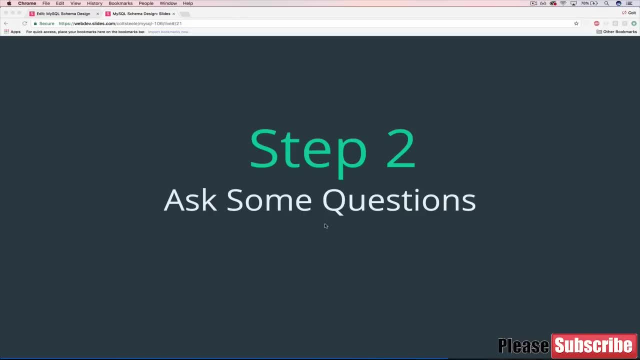 else and you have to use some- most likely anyways. So that's how we're going to work here, And we'll start out nice and simple in this first video. Suppose that we want to reward the users who have been around the longest, So you may have seen something like this on Instagram. 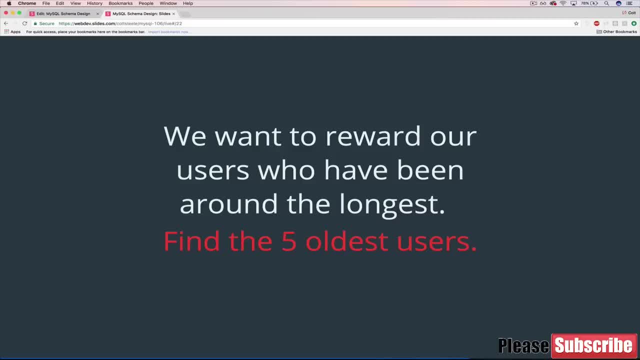 Other applications. you'll sometimes get a coupon or just a thank you email, Thanks for being loyal over our five years or however long we've been around. So all we want to do is reward our users who've been around the longest, And to do that, we need to find the five 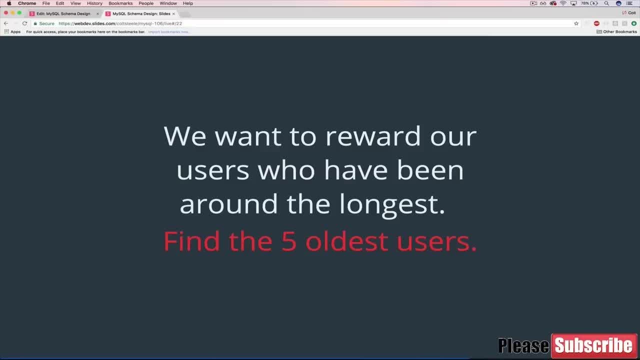 oldest users, the users who have been around the longest. So this one is should be simple, not crazy. We don't need to work with many tables. Short video: Try this on your own. Pause the video, Of course, And in like three seconds I'll be right back. 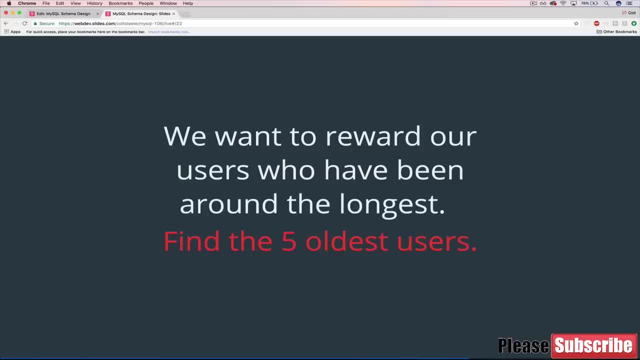 And I'm back So to do this. it's just a matter of basically selecting star from users, And then we just want to order them based off of the date that they were created, the date they joined, And then we'll limit it to five. 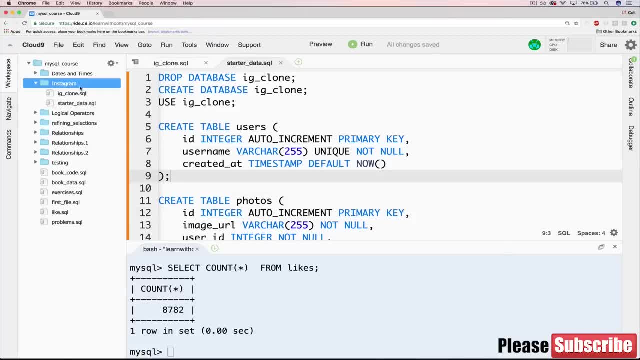 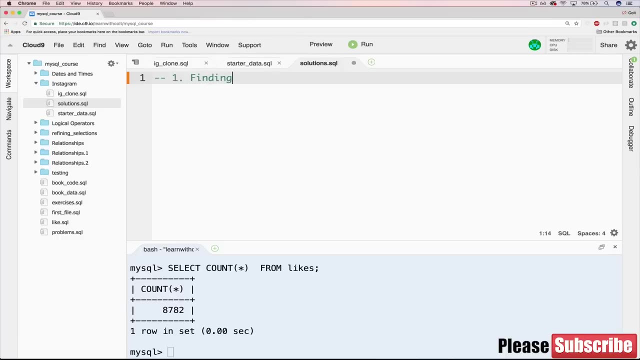 So if we hop over, what I'll do is make a new file, New file- where are you? And I'll just call it solutions, dot, SQL. And in here, the first one is just finding the numbers here, So it's easier for you when you're looking at this. 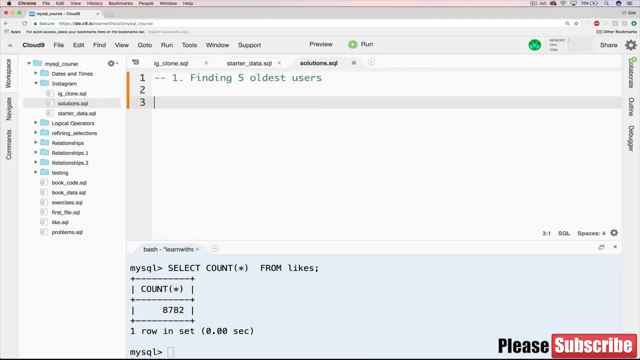 Finding five oldest users, And we know it's going to be a select, something from users- And if we start there, you can see we've got 100 users, which is one thing I wanted to point out. 100 users is not very much, but I capped it at 100 because 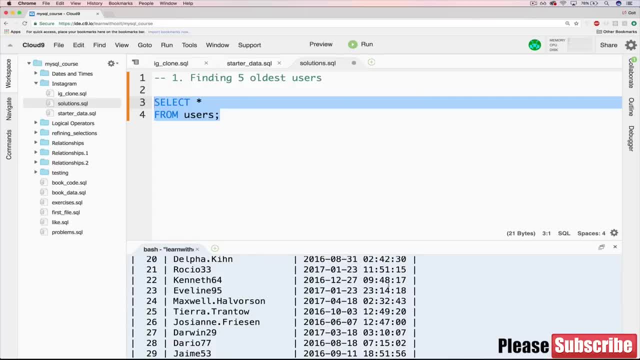 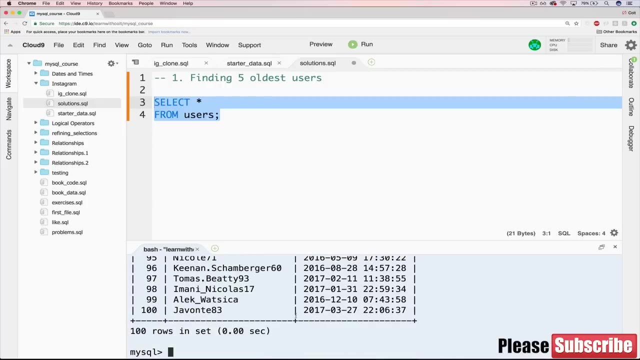 basically the formula that I imprecisely came up with for how often users are commenting and posting and liking and tagging. it grows exponentially depending on how many users you have. So, having 100 users, we still have almost 20,000 records for everything else. 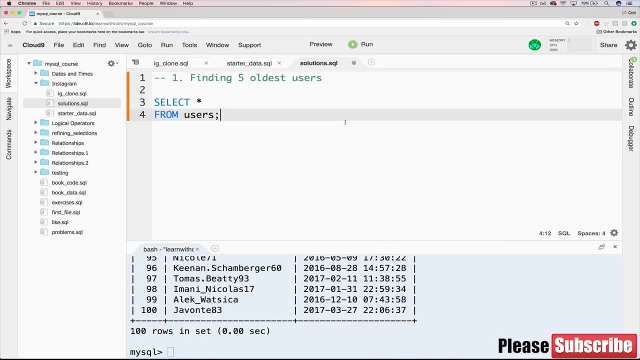 And if I upped it to 200 or I tried 1,000 users, at one point it really started going crazy and our queries take a lot longer. So I decided not to do that. But if you want to try, it could be fun to, if you feel comfortable writing code. 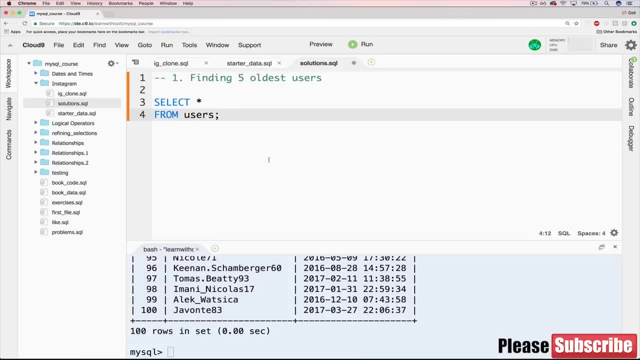 to insert a bunch of users. do that in JavaScript or Python or whatever language you like, but for now 100 users. it's just interesting to note how much data we get even with just 100 users, if the average person is posting, you know. 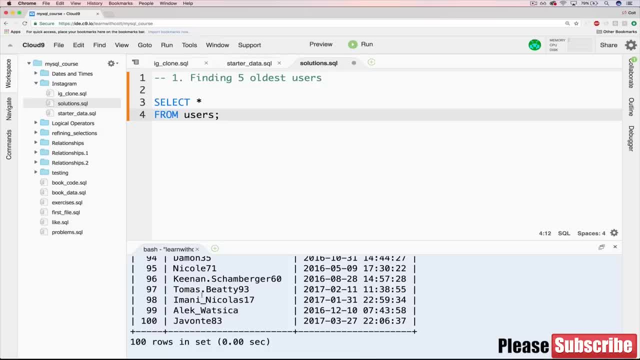 X number of times. and then we get certain celebrities who post all the time, not to mention people who are liking all the time, and we get bots who like every single photo. things quickly grow OK, so select star from users, but we want to order by. 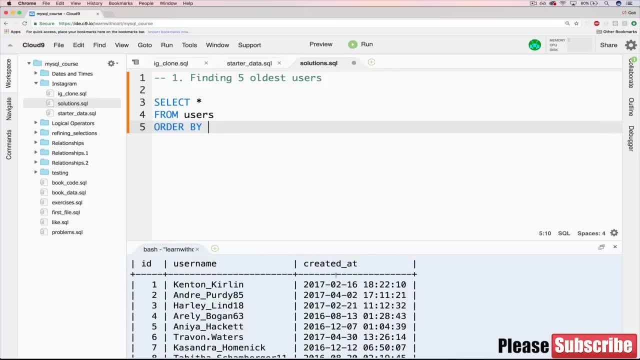 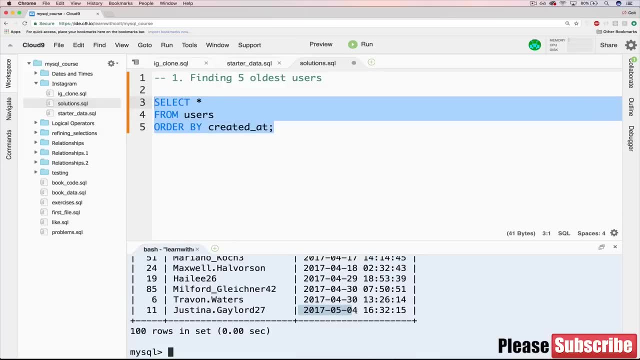 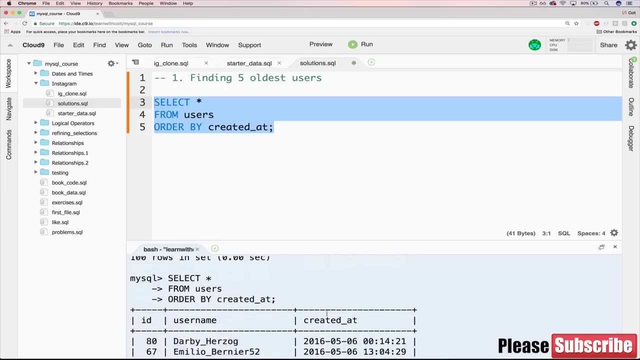 and our field is called created at, Right there. so just order by created at. and if we just do it this way, you'll notice that at the bottom we have today's date, basically roughly today's date, And then, if we scroll up, 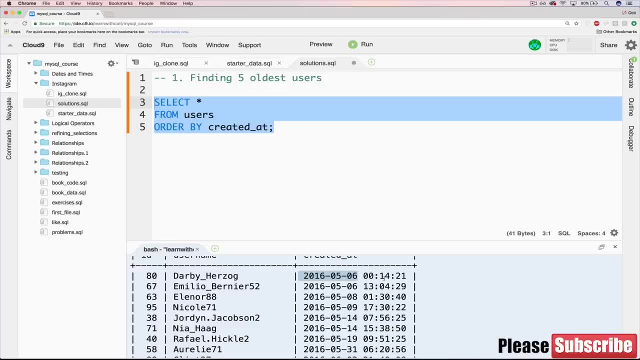 We've got the oldest one, so we've only been around for a little bit- about a year, according to the data that I created. So what we'll do is just limit five And there we go. that's all we need. 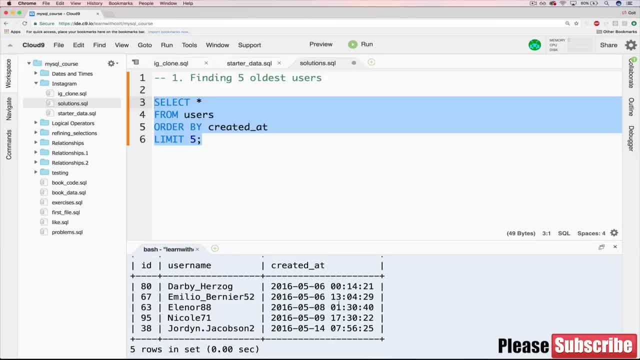 So nice and simple for this one. I want to start off with some review, but don't worry if this felt way too easy, That's OK. that's good. We're going to move on and get into some more exciting slash, potentially nastier territory. 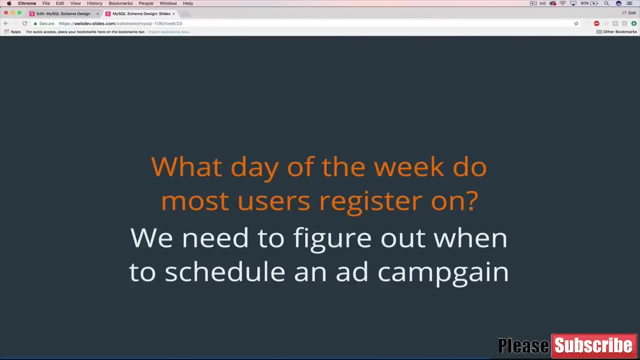 All right, All right. So the next problem here, the next question, is that we're trying to schedule an ad campaign, our own internal campaign That we're going to- well, not internal, but our own campaign where we're trying to get people to sign up- new users- on our application. 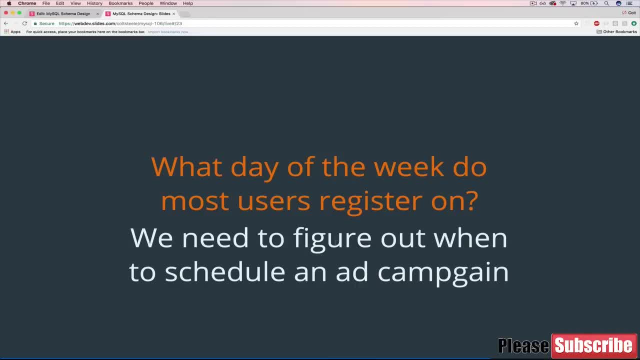 Let's say we're advertising on Facebook. We're also considering, maybe for a single day we're going to go and put an ad out like on a billboard. We can't afford a billboard for an entire week, so we're just going to do one day. 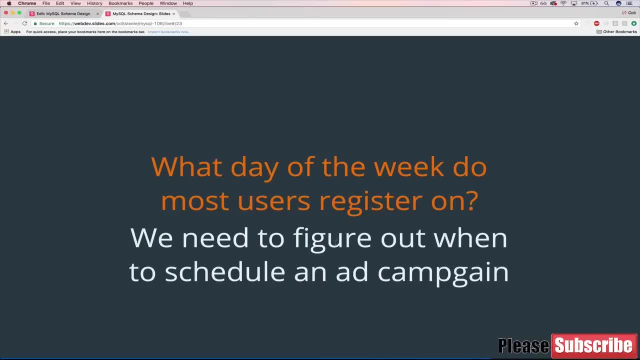 Yeah, it's kind of hypothetical, but still let's say that's what we're working with. And you could expand that obviously to whatever the budget is and whatever your constraints are. but for us, low budget and we're just going to run an ad for a day. 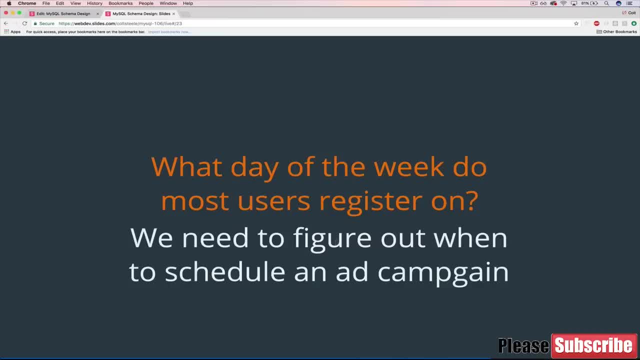 We want to figure out what day we should do that on, what day of the week is going to work the best. This is something that is definitely relevant, even though it's simplistic. here We're figuring out, you know, days of the week or time of the day. 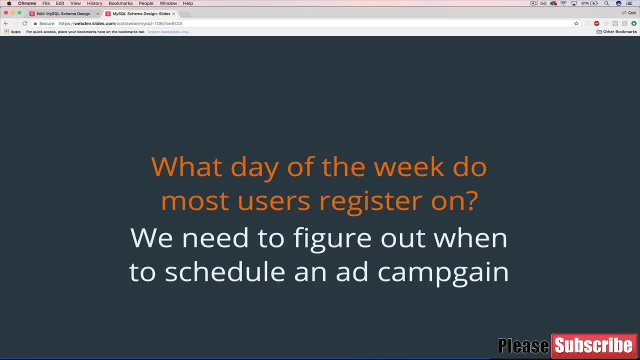 Just as a photographer. that's something that is useful. that people are always trying to figure out is what's the best time to post something on Instagram. What's the worst time? What day of the week is the best Do you wait? for? what time zone do you try and post according to? 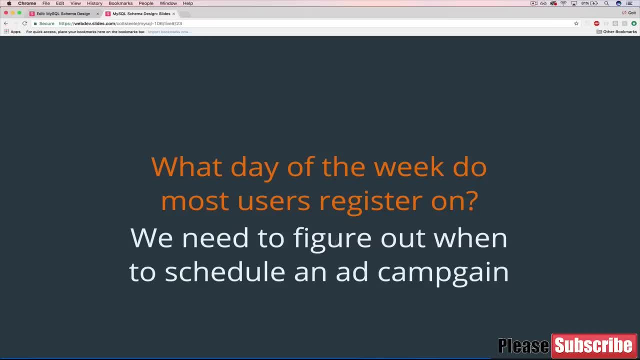 Do you post something so that people in Europe will be able to see it when they're waking up? There's this whole science, and that's just for photographers on Instagram, who are not even really making any money from it. So if you start thinking about advertisers, then that's where it really matters. 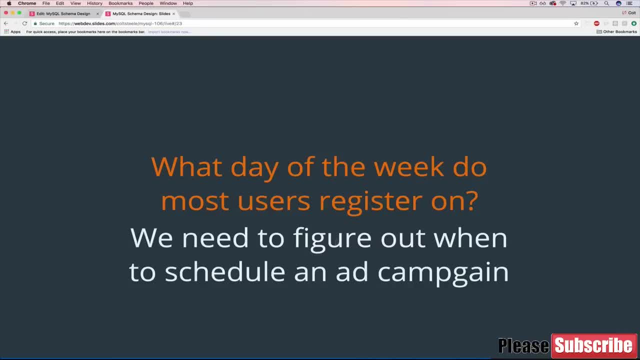 So we're just doing this simple thing to figure out when users register. But there's all sorts of insights to be garnered about when people are posting photos and how many likes photos get, depending on what time of day they're posted, and all that kind of stuff. 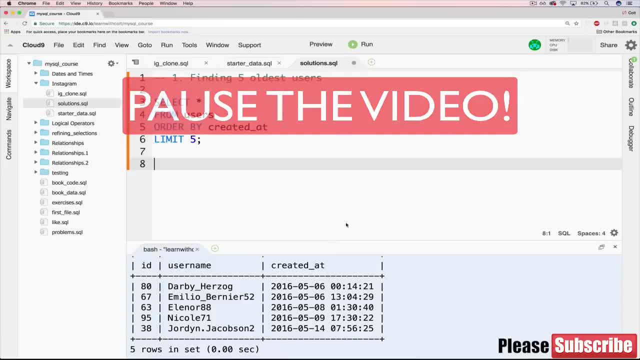 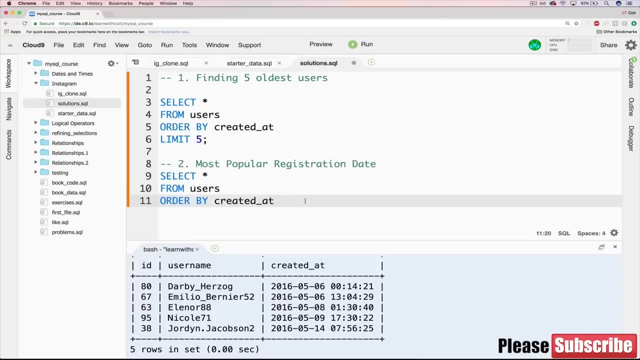 But we're working with this. So what day of the week do most users register on? So we only need to work with users still. So I'm going to just add a comment: Most popular registration date- So we can recycle part of this query: select star from users. 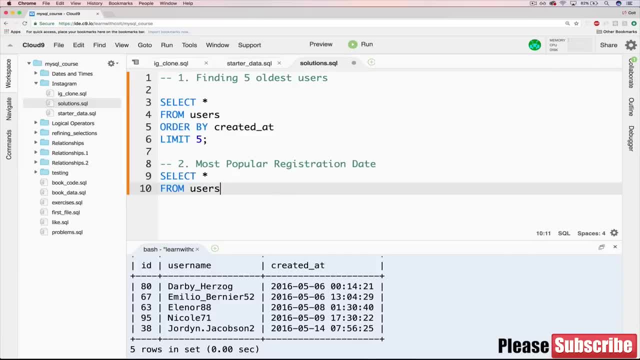 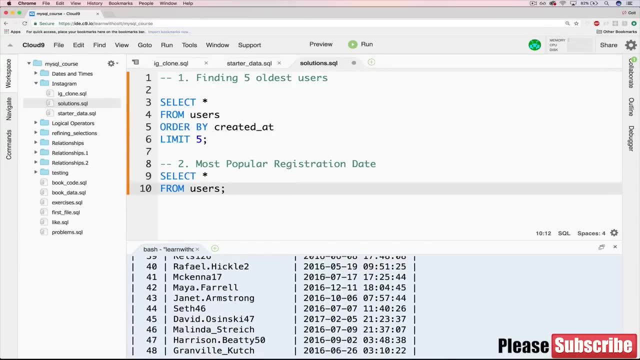 and we don't really need to order by anything at this point, so I can get rid of that. So what we want to do is use a group by to collapse these into similar categories, But we can't do a group by created at, because unless somebody 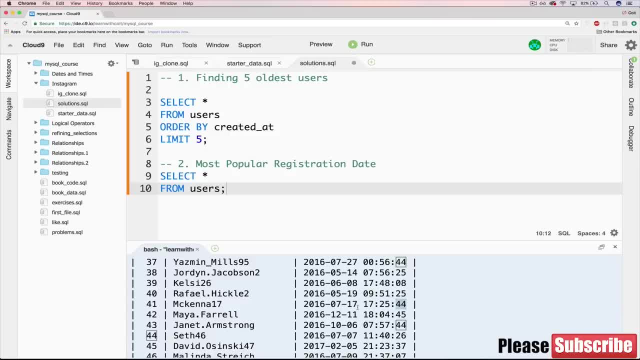 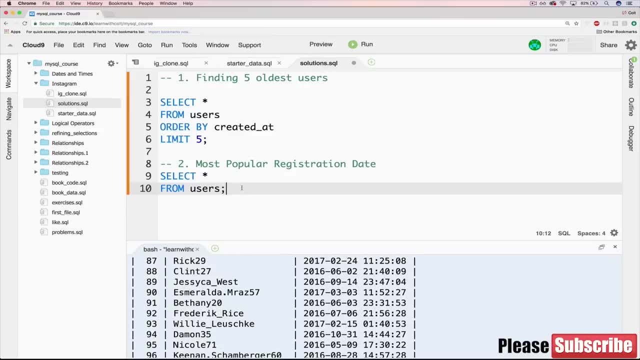 registered at exactly the same time down to the second on the same day group by won't work and it will just have 100 unique users. So what we can do is basically extract the day of the week, which we've seen how to do that. 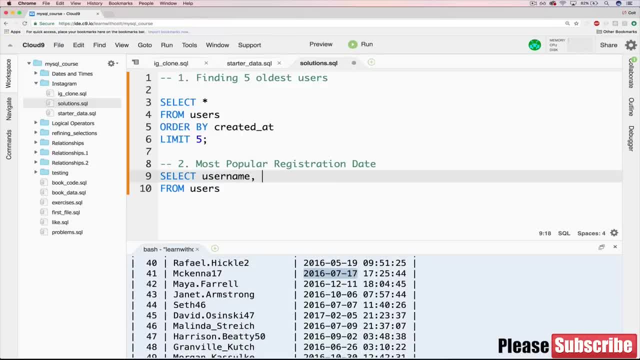 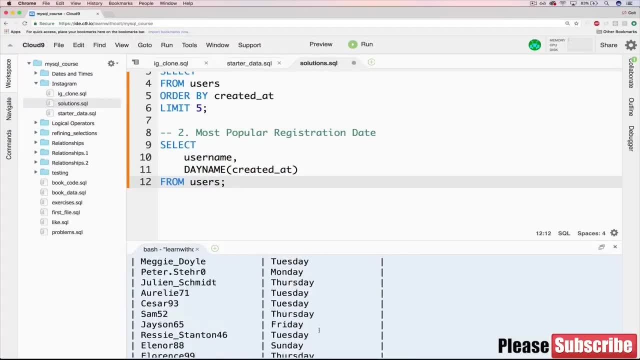 So let's start with that. Let's just do select username comma, and I'll do this on separate lines: Username comma and then we want day name. This is one way of doing it. You could also use format date. 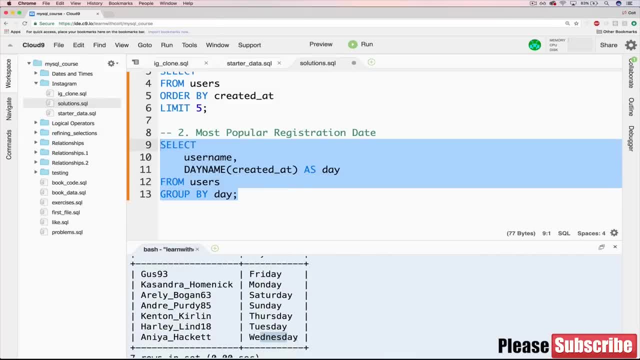 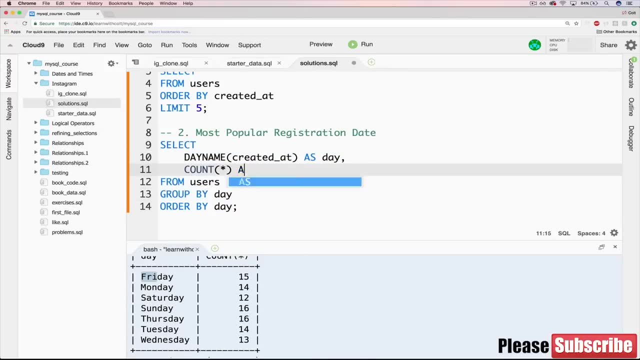 but day name. I happen to remember that one, although there are all those other methods I don't remember that are functions I don't remember that I've talked about like the name of a month. I always forget, So sometimes I do end up just pulling. 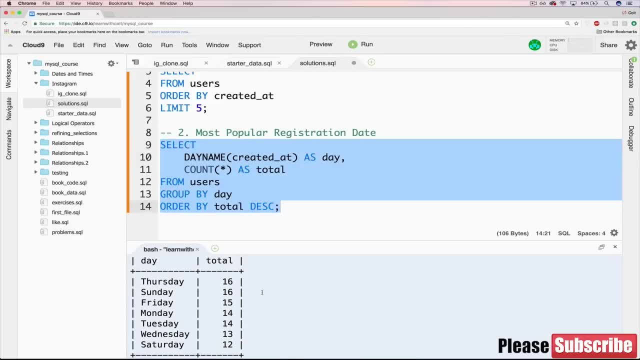 open the docs and trying to find the right function, But day name, and then we just pass in created at. OK, Let's try that. Oh, semicolon, before I forget that. So now we're seeing the day of the week, So now all we want to do is group them. 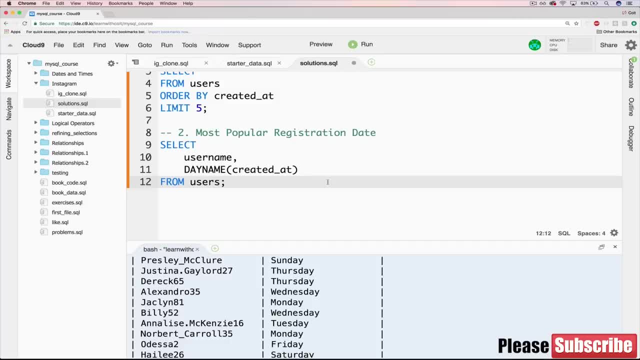 By those days of the week and then count how many people or how many instances we have for that day of the week, And then from there we'll just order them to figure out what day is most popular. OK, so rather than just doing this, we'll add our group by at the end. 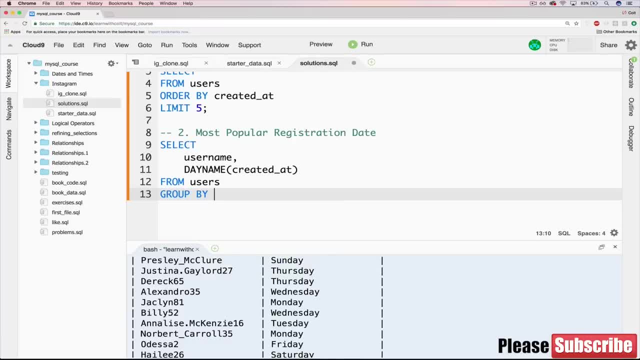 And we don't want to just do group by like a group by created at. Like I said, we want to do a group by day name created at, And what we could do is just assign an alias here. So we'll just call this day. 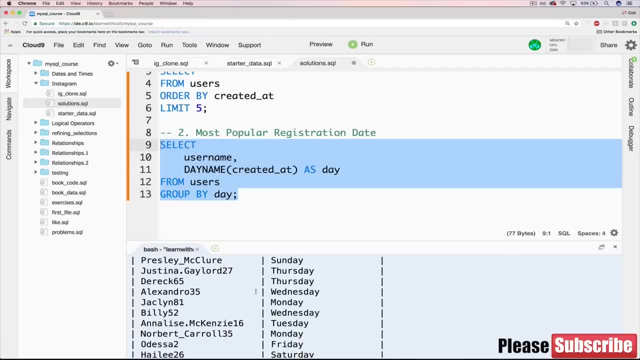 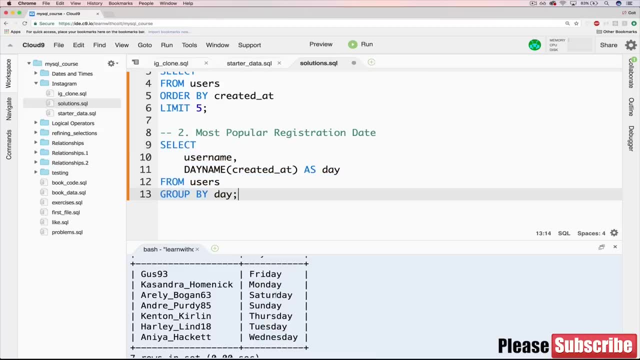 And we can just say group by day. Now, if I do this, I only get seven results: Friday, Monday, Saturday, Sunday, Thursday, Tuesday, Wednesday, And of course that's not all the data. that's there, That's all that's printed out, because these groups have been created. 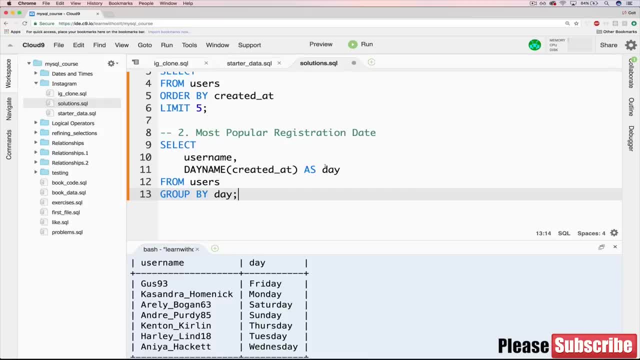 and we can work with them behind the scenes or underneath the surface. So what we'll do? we can get rid of username at this point. We don't care about that. We're going to just group them by day and then we're going to add our count. 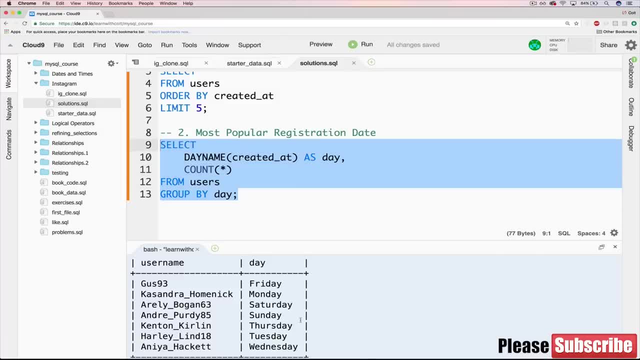 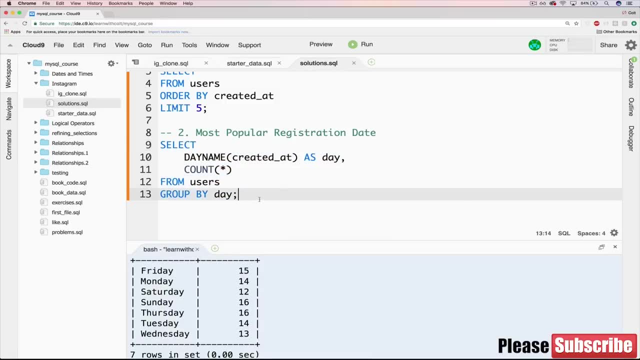 Star, just like that, And let's see what we get. OK, so you can see, it's a pretty even distribution. Let's go ahead and sort, So we'll do an order by day. Whoops, we don't mean day. that's ordering alphabetically over here. 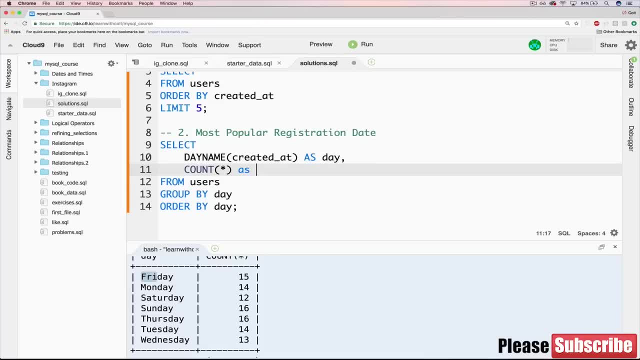 We want to do is order by count star, So I'll give that an alias as well. I'll call it total. We want to order by total, All right, And of course, if we wanted to, can change the order Technically. the question we're asking is: what's the most popular day? 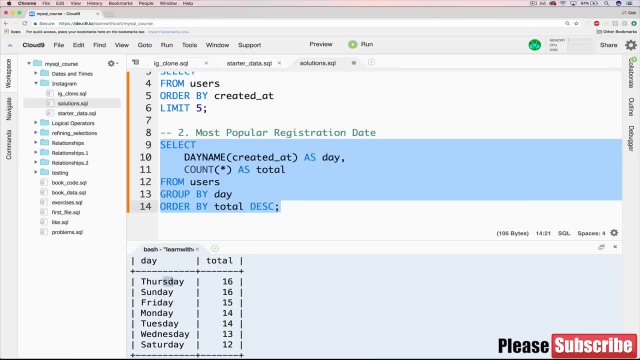 And well, we actually have two days that are tied for that, Thursday and Sunday. Now this data is not relevant to the real world. I have no idea. Actually, I'm pretty sure those days are not the most popular. Last time I looked into it for my own purposes, I believe. 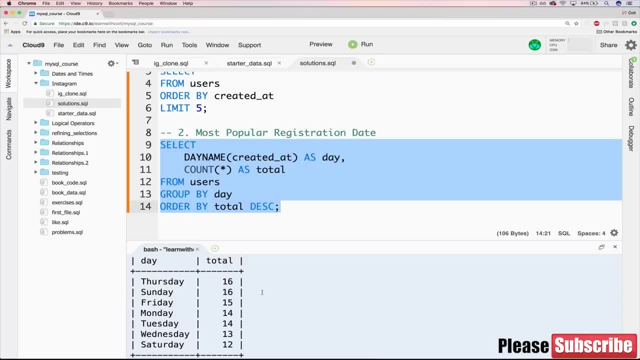 Oh boy, I believe it was the middle of the week, like Tuesday and Wednesday, roughly late afternoon, early evening Pacific time, like five pm Pacific time is the best time. I'm not sure why, but again, I didn't create this data to be realistic. 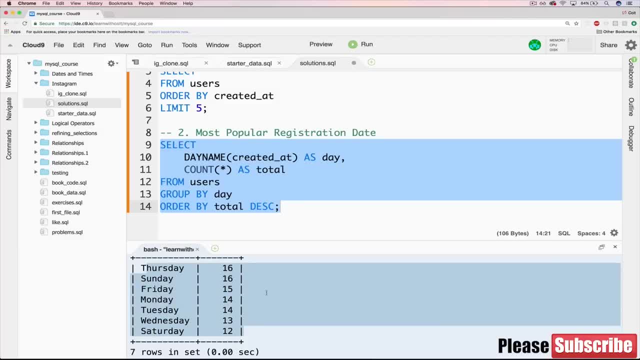 I just tried to come up with something that would be interesting, whether or not it actually applies to the real world's rules. OK, so what we could do is, you know, limit it at the end If we just limited it to one. 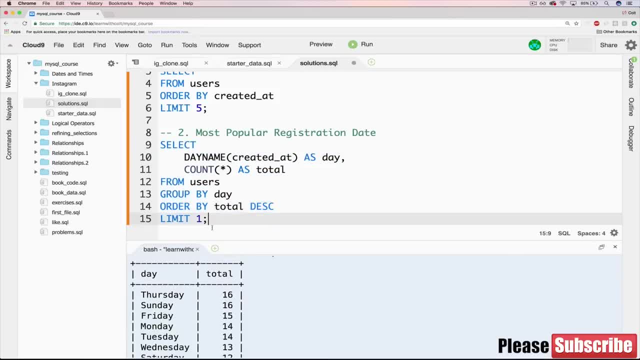 It gives us Thursday because it comes first. We could do a limit to as well. All right, and this is a good time to mention that for most of these things in this section, there isn't only one way of doing it. Sometimes there really is. 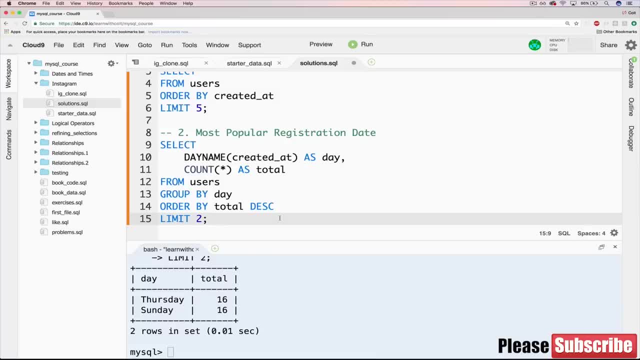 But often there are a couple of different ways of approaching things, And if you feel like you came up with something- whether it's just different and you're not sure if it's better, or you feel like you did come up with something that's more efficient or cleaner, or that you 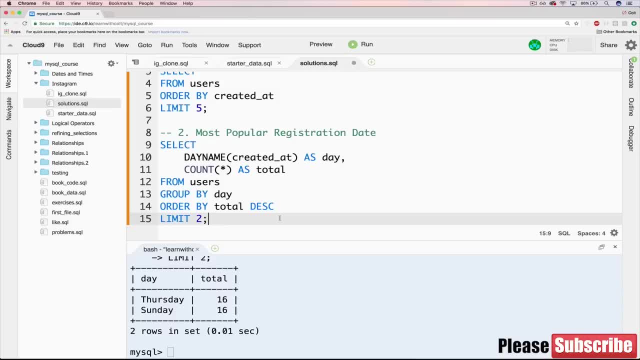 prefer. absolutely don't hesitate to post that in the discussion for the course And we'll do our best to get back to you with feedback on it. But at the very least other students will be able to see it And maybe somebody else came up with the same thing and they won't feel so alone. 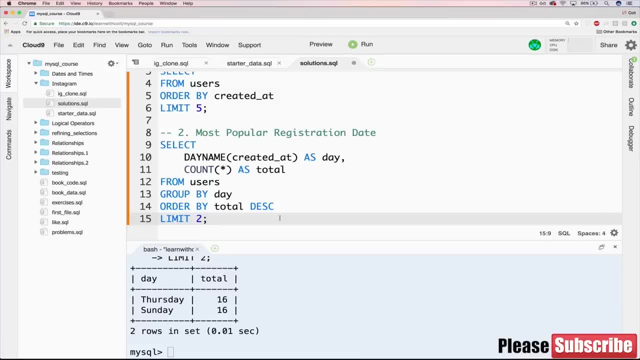 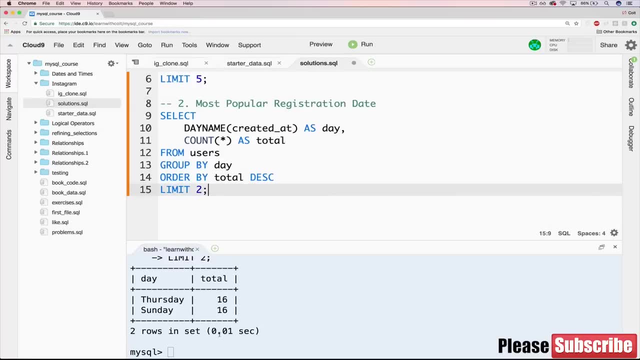 in the world, Or maybe you did come up with something better that is actually going to benefit other people to see, But for now this is how we're doing: most popular registration date And that answers our question Apparently we should be doing. 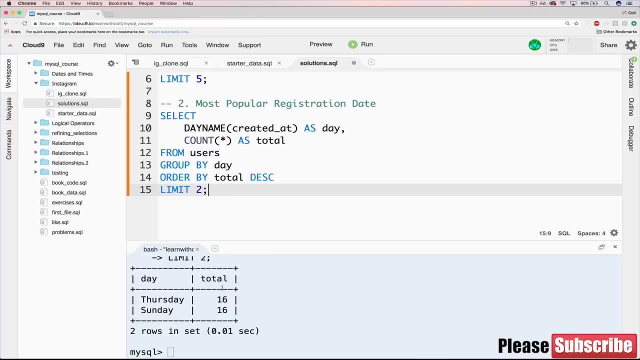 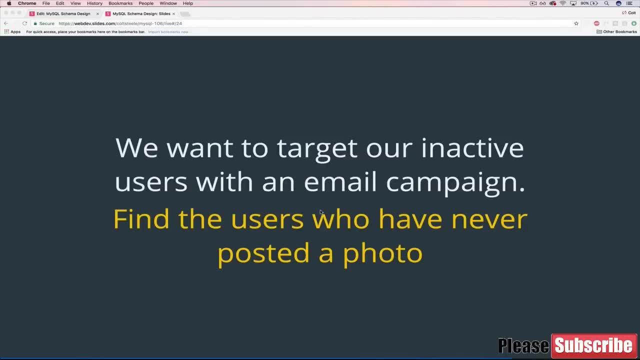 our registration campaign to get users to sign up on a Thursday or a Sunday. All right, Welcome back. So we're moving on to our next question here, even though this one actually isn't framed as a question. there's no question mark. 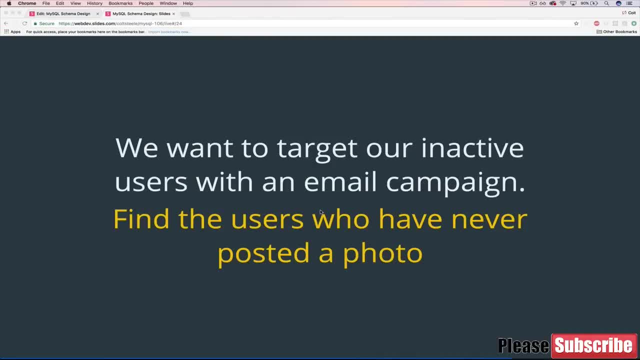 But that doesn't make it any less relevant or less real world. In fact, this is one that I think is a really common operation, a common question to ask, And it has to do with inactive users. So, across any sort of startup or online app company, there's often, you know, users. 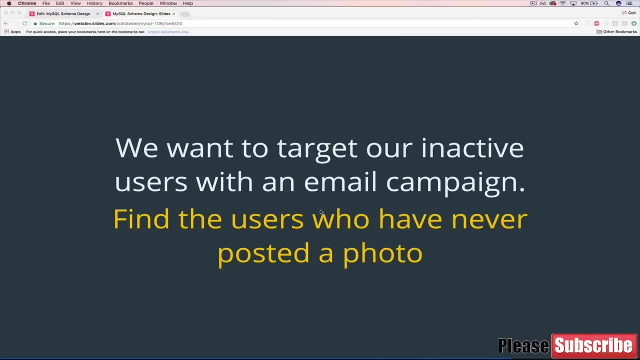 who sign up, create an account and then do nothing, whether it means never posting or never buying something, never converting from a free account to a paid account, like in the case of Spotify, or never In my case. you know, this is a real example for my courses. 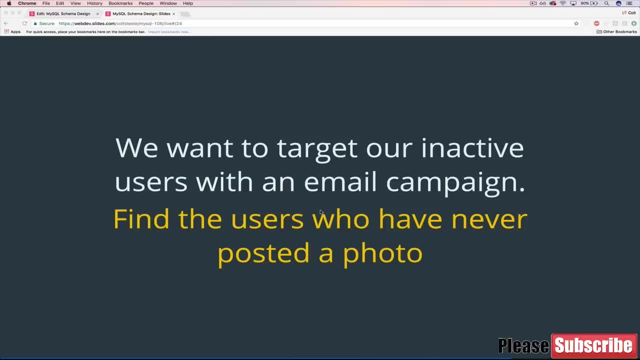 students who sign up and then never start it, never make it past the first video. They're at zero percent And I'm actually able to send targeted, I think once a month, twice a month, I can send an email update and I can target that. 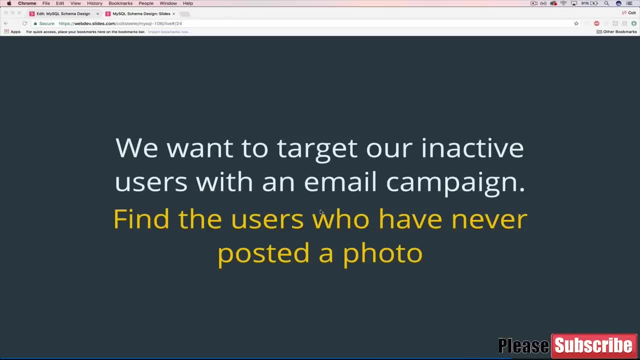 To specific segments. So if I updated an introduction section to a course and I only want to let students know who haven't started yet, I want to target them and say: hey, by the way, I notice you haven't started yet. Well, this is a good time to start. 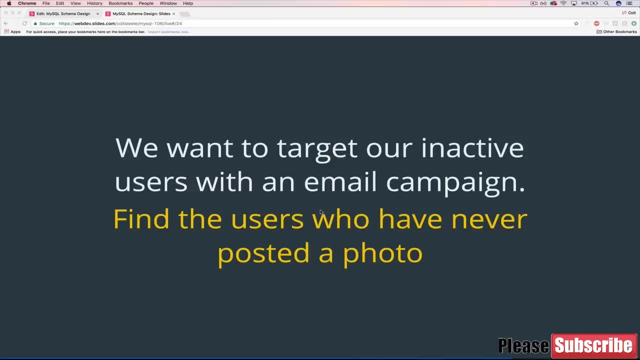 I just revamped the whole intro. I could do that based off of what we're going to be doing here. Of course, our data and our database is set up differently, but it's the same idea, So this is a really common thing. 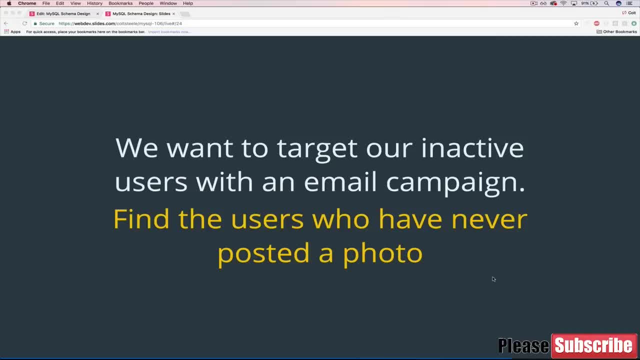 And all we're going to try and do is for our Instagram clone, our fake Instagram. we're trying to identify users who have never posted a photo. So they've signed up. They never posted anything, And we want our users to be more engaged for a bunch of reasons. 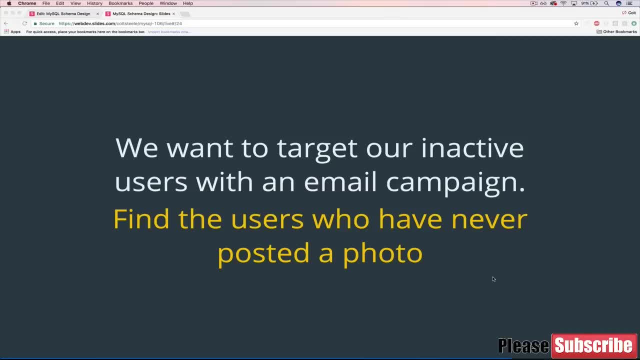 You know, we want higher engagement in our app, which means that we could have higher valuation potentially, or sell ads for more, maybe get higher investments- all that kind of stuff We want people posting if they're signed up. It looks bad to have dead accounts, people who sign up and then give up. 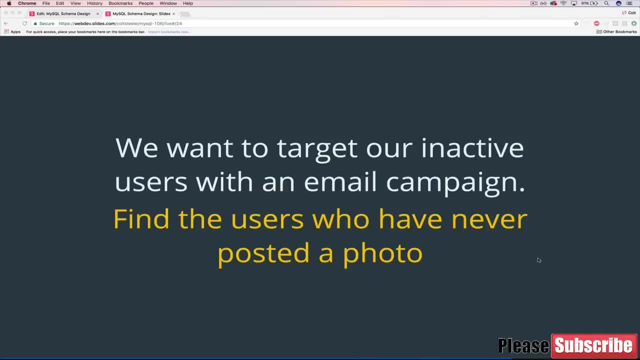 So we're going to try and send an email. We're not worrying about doing that. But how are we going to target these people who have never posted a photo? First step, let's identify them And essentially, we're going to need to work with the users table and the photos table. 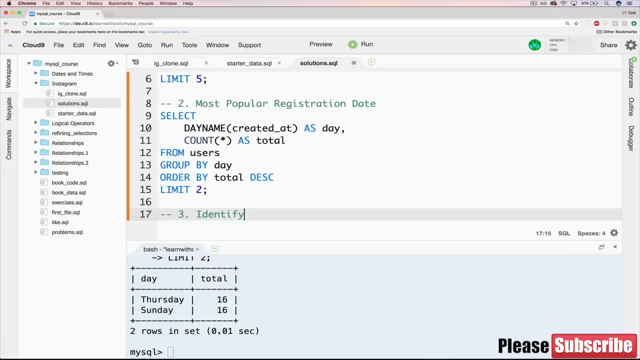 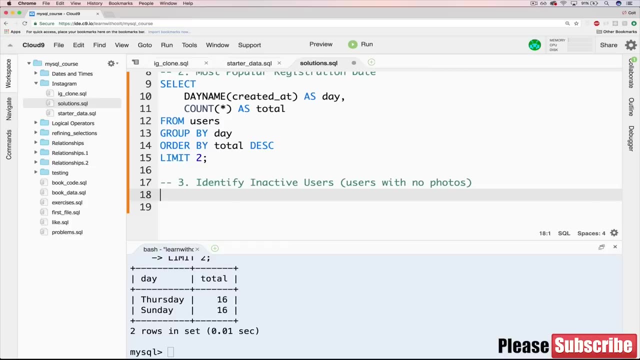 So I'll add my three here, which is identify inactive users, users with no photos. OK, so you've probably gathered we need to do a join. We're going to be working with the users table so we can start there. So we're going to select star from users. 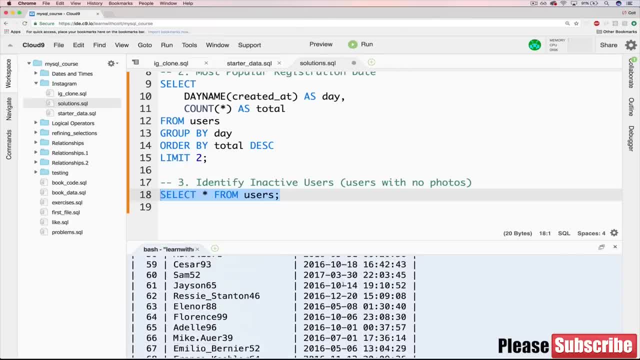 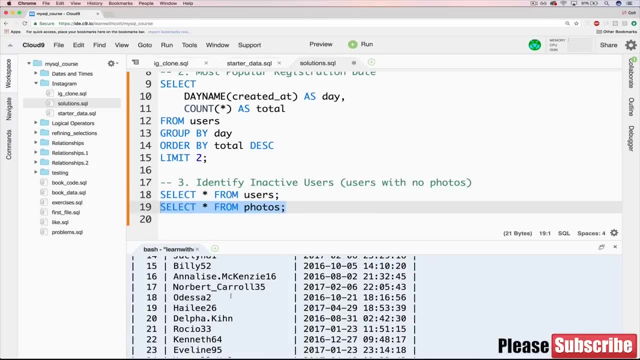 And you know we have one hundred something users but we can't see who's done what, because we have the photos table And if we do our select star from photos, just to jog your memory, Well, I guess we haven't actually seen all of our data here yet. 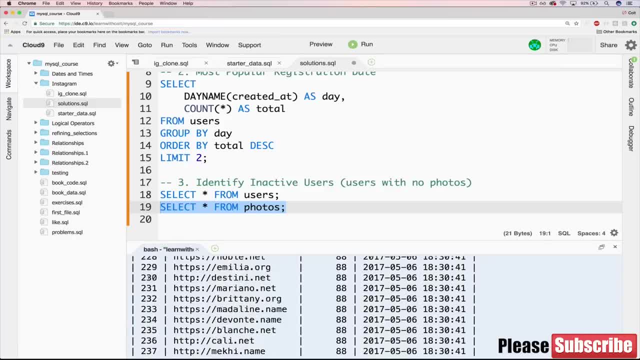 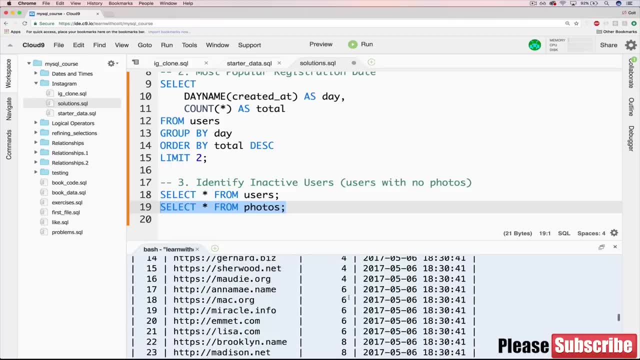 We've got about exactly two hundred and fifty seven photos, but a lot of them are done by the same user, So this here is user ID. If I scroll way up, here we go, we can see, you know these these are. 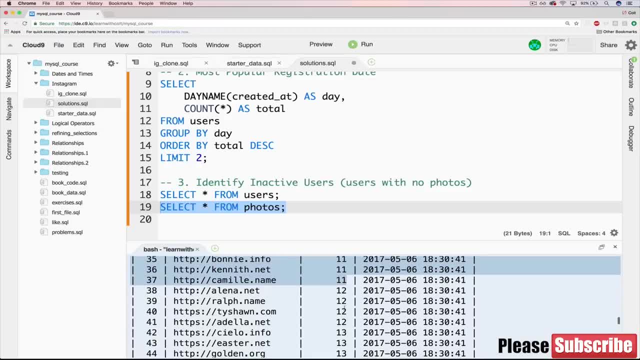 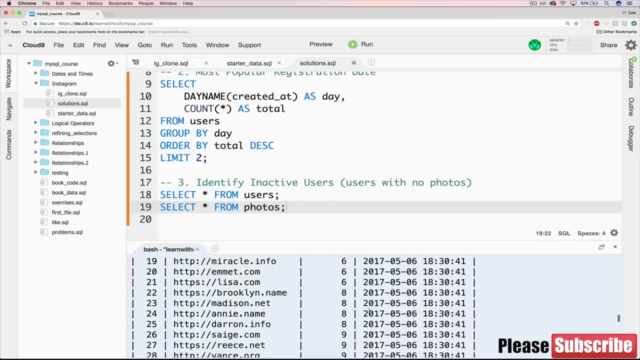 all posted by the same user. So three These are all from the same user. These are all from the same user. But then we have some users who haven't posted anything. But there's no way of knowing that, just by looking at the photos, because these are the posted photos. 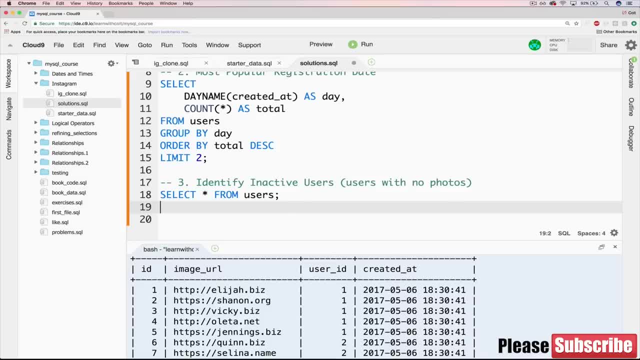 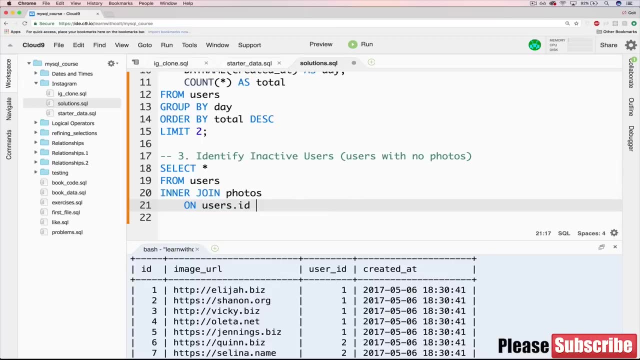 So what we need to do is join these two together And hopefully you know what we need to do. If I just do a regular inner join, Inner join photos and where we want to do it on a join on users dot ID equals photos dot user ID. 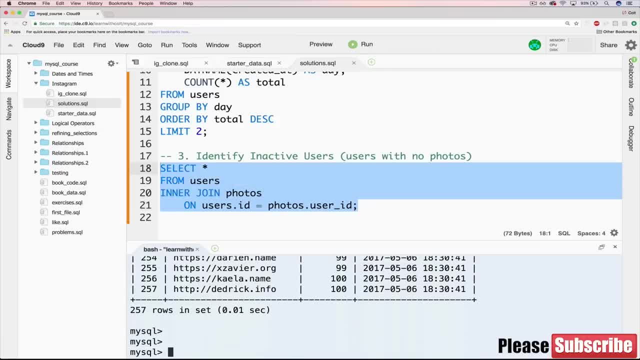 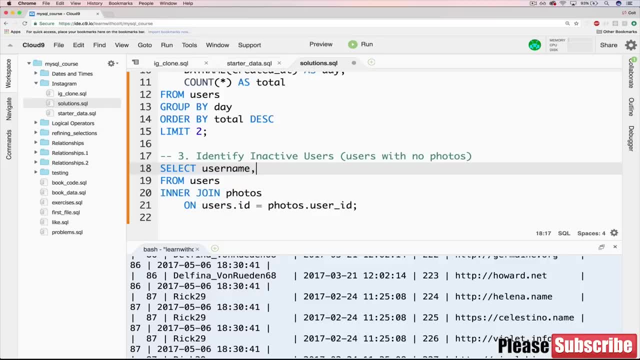 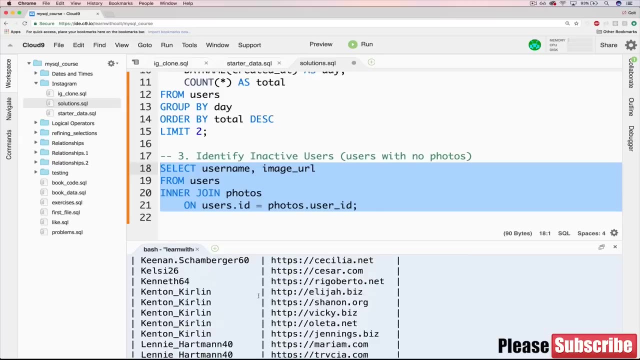 And if we run this now, It's a mess, so let's focus on just the things we need. So, rather than star, you can do username, maybe the image URL, and we can just start with those two, All right, so we can see all these usernames and what they've submitted. 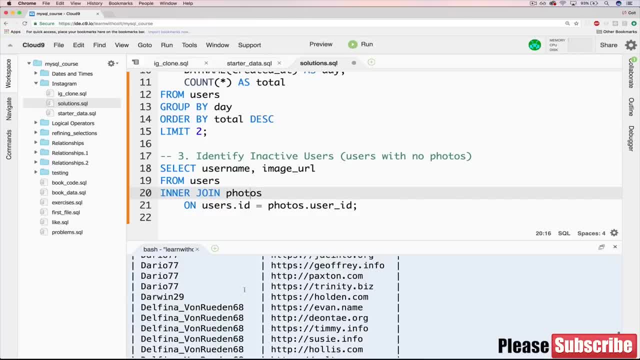 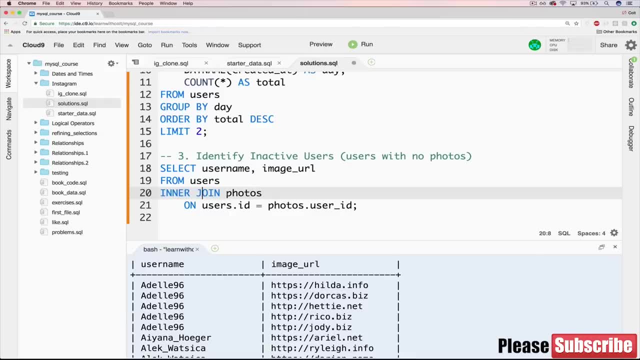 But the problem here is that this doesn't account for the people Who haven't submitted anything. So if there was a user who didn't submit something, they're not showing up here because we're doing an inner join which, remember, is the intersection of both. 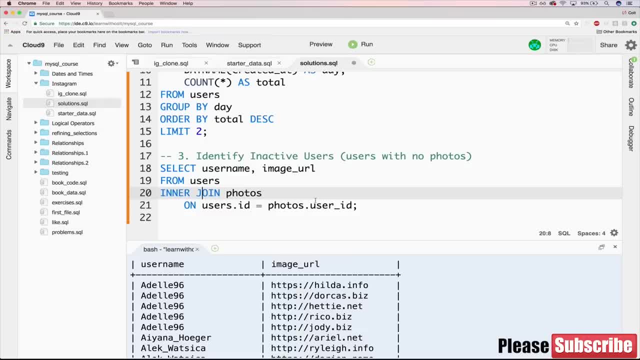 circles the left and the right where they overlap. But what we want is to identify where users on the left have no overlap on the right for photos, So we can change this to a left. join in that one change. We rerun this. 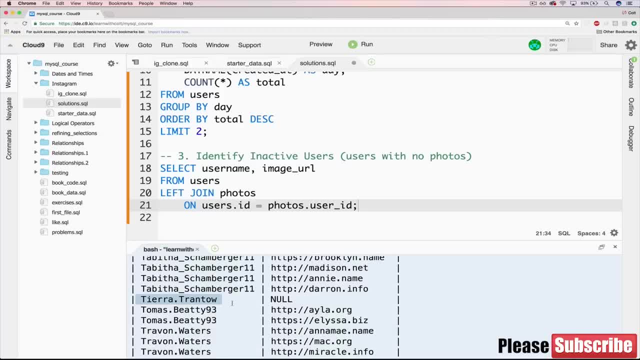 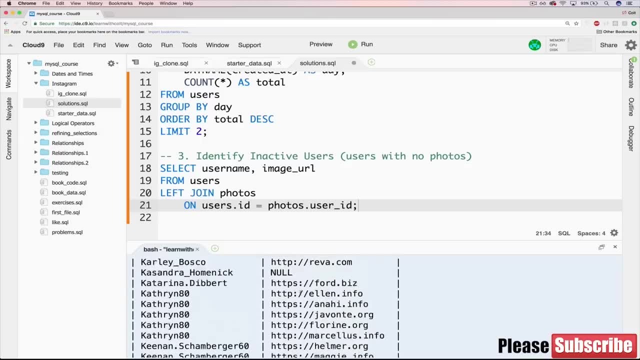 We'll have to scroll a bit. There we go. You can see we have certain users who have a null over here And that's referring to the fact that they have no photos corresponding to them. So there's a couple of them as I go here. 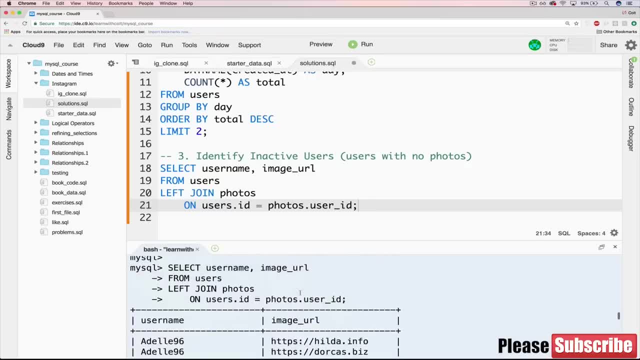 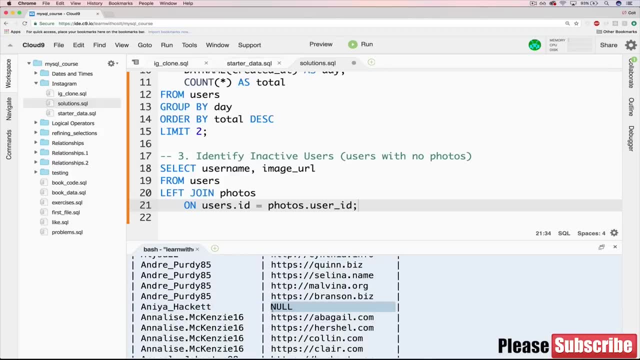 And that's what we want to be able to identify. So we're almost there. actually, All that we need to do is only select the users that have photos of null. essentially- And of course, if I go back to having star here, it's not just image URL, that's null. 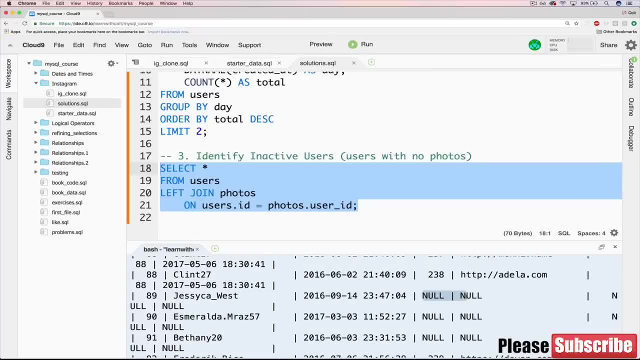 It's everything in photos. It's hard to see. Here's an example. But we've got a couple of nulls here. We've got the image or the photo ID, We've got the image URL, We've got the user ID of the photo. 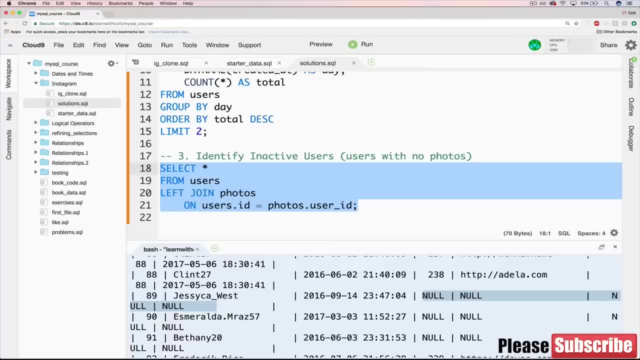 And then we have the created at is null. So all four things are null. We just need to focus on one of them. It doesn't matter which one, So I'll go back to just adding username here, and we can do It doesn't matter really. 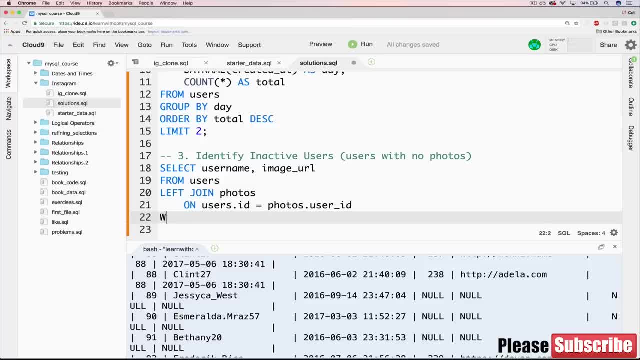 Let's do image URL again And then all we want to do is add a where down. But we can't just say where photos dot. we could just do ID equals null. That doesn't work, Remember, null is weird. So we need to do where photos ID is null. 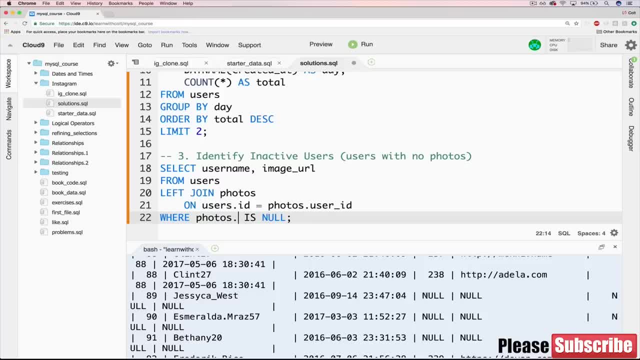 And this could be anything on the photo side. It could be photos that ID, It could be photos that image URL, photos that user ID, any of them. So I'll just do it as ID And if I do this now, you'll see, and we actually don't even need. 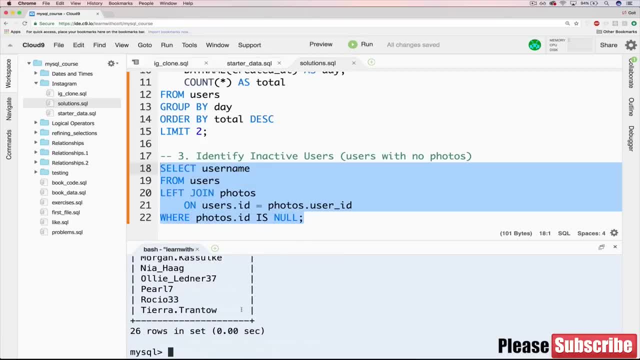 to display the image URL, but if I do that, This is our list of users who have never posted anything for whatever reasons, some of them programmatically. I created them as bots which all they do is go comment and like other people's photos, but they don't post anything themselves. 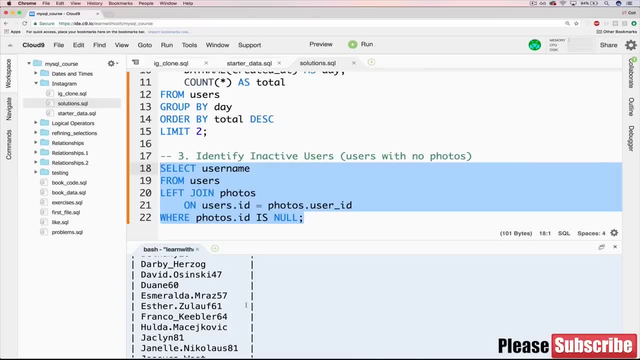 And then another persona of a user is a lurker, which is somebody who has an account and they don't use it all that much, but they just kind of look at people's photos, maybe like something, But they don't really. they definitely don't post and they don't comment. 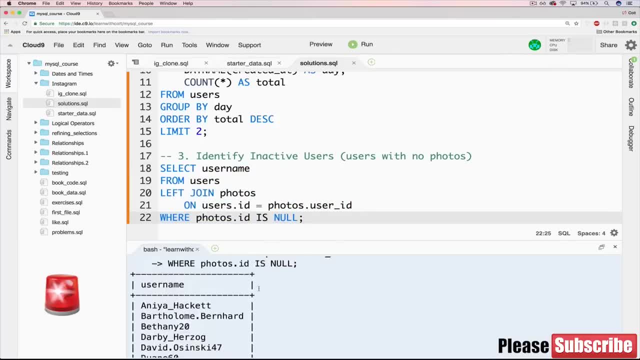 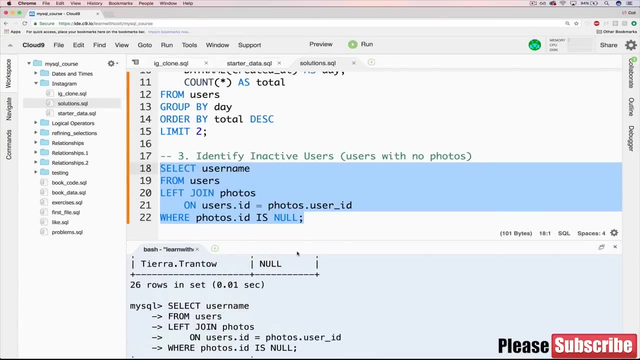 They're kind of a silent member of the community, So we get a decent number of them. Sorry for that firetruck And that's all we need to do If we want to figure out how many. that's another thing. we can just add account in. 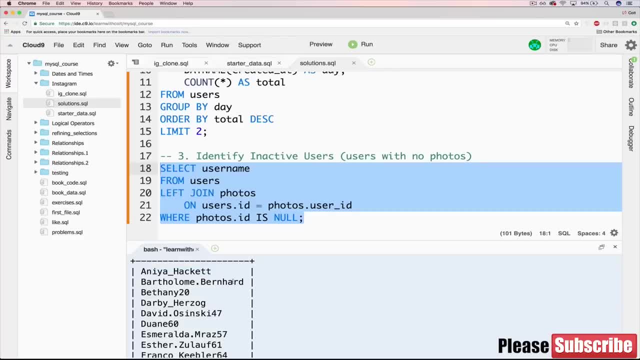 But you just want the username so that we can target them. These are people have never posted anything, And just a note. you know, if you did this the other way around, it would have worked just fine as well, to do photos users and then a right join. 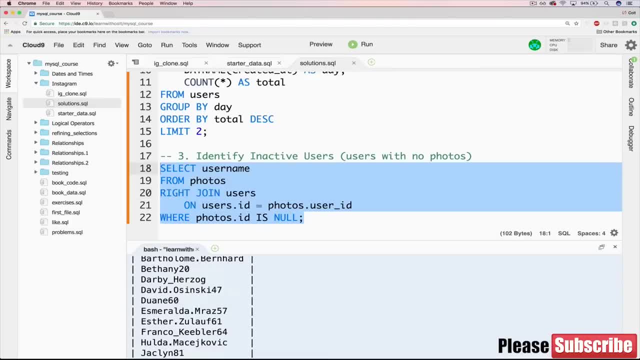 It does the same thing, So either way works. But the key thing is that we are working with null, where we have an intersection where some users and some photos overlap- Most of them do, But then we also have that subset of users who have no photos. 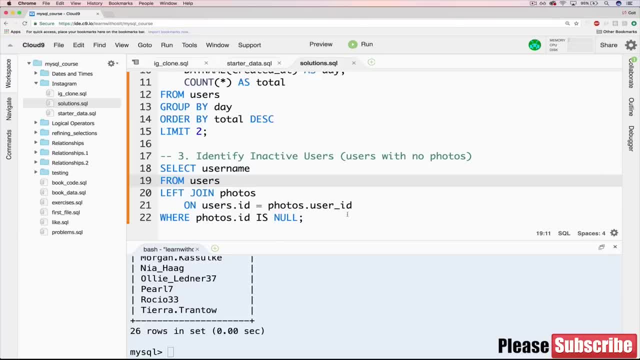 And we need to also join those with null, which is how we were able to tell if they have no photos. So here's my solution. You came up with something different? post it and we can discuss it. Moving on, Alrighty, welcome back to our next. 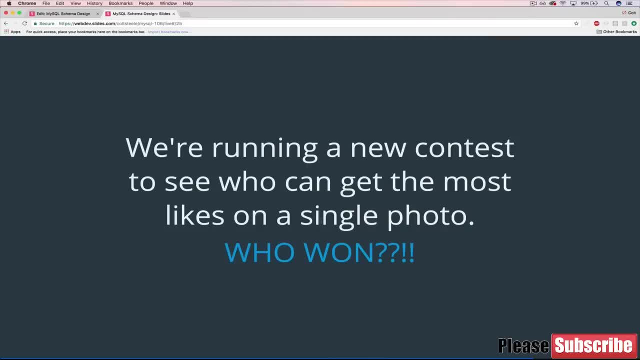 riveting installment of asking random questions about our database data that we inserted. Yeah, that's, that's what we're doing here. So our next question here is basically- I'll start the other way around for once. What we're trying to do is figure out what 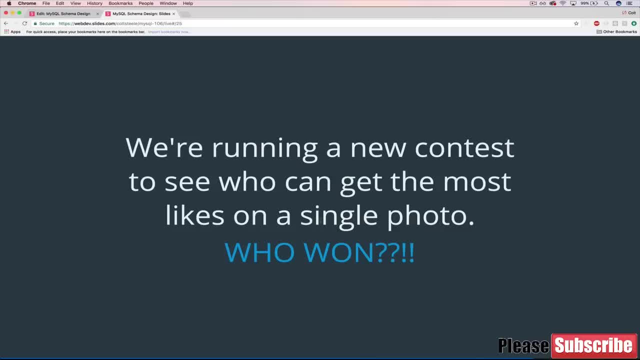 is the single most liked photo in our database And I actually don't know if Instagram has done this before. I know third parties have, like people have used Instagram API to try and find out the most popular Instagram of all time. That's essentially what we're trying to do. 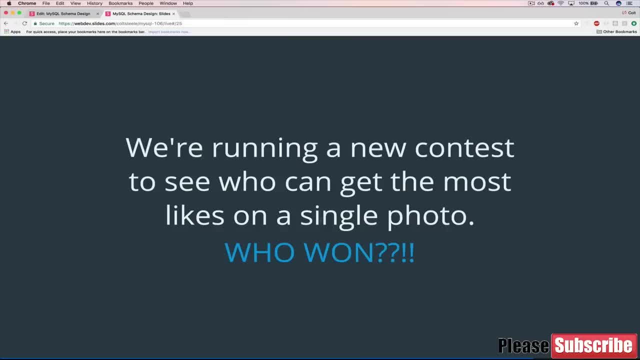 Let's say we're running a contest- is the back story I came up with, But this is something that just might be nice to know internally at a company like Instagram, who is responsible for the most liked photo of all time or the top ten most liked. 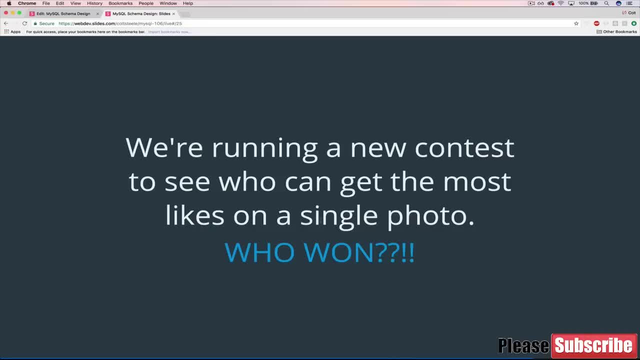 Is there anything in common? or even the top one thousand? What ties them together? We're doing just one, and we're not just trying to find the photo itself, but we all know who posted it, who is responsible for it, So we can send them, whatever their prizes. 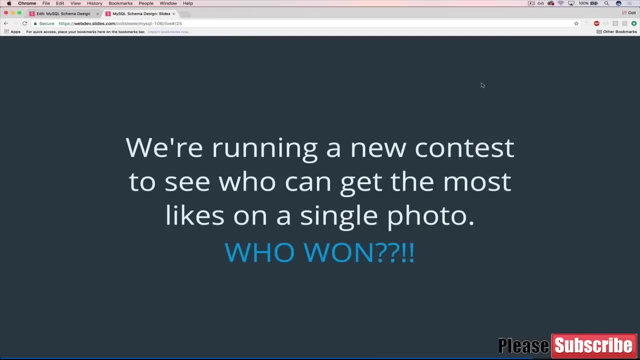 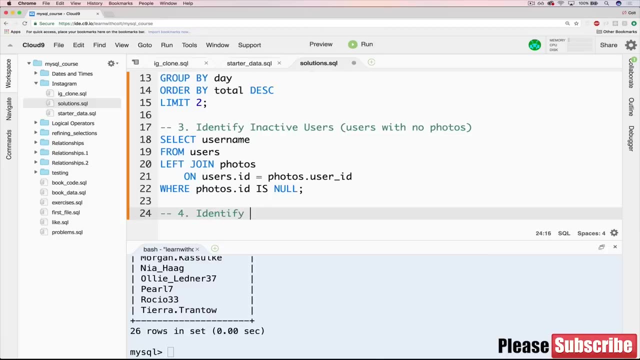 or we can mention them in a blog post or something. So the first thing we need to do is just find the most popular photo, to start meaning the most number of likes, and then we can worry about the username and the user afterwards. So we'll do for identify most popular photo and user who created it. 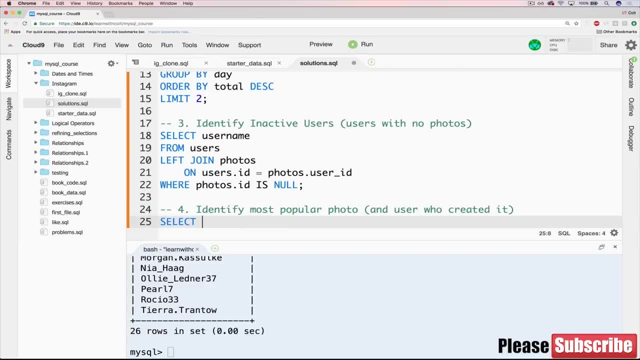 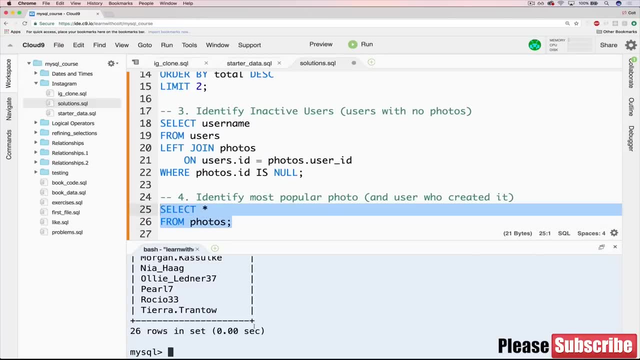 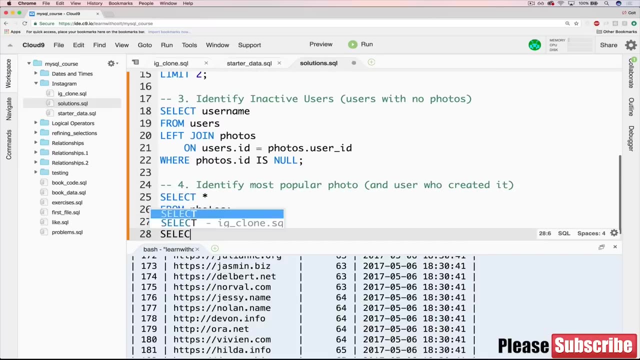 OK, so to do that. it's going to be a select. we'll do select star to start from photos. And if we just start there and we have, what is it? two hundred and fifty seven, but no information about likes, because that's a separate table. of course we do our select star from likes. 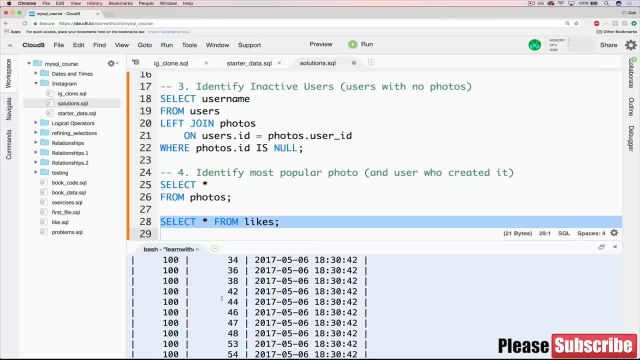 We have eight thousand seven hundred and eighty two likes, and they're not all displayed here for us to see, but we've got two fields. we have the ID of the Person who is liking the liker, and then we have the idea of the photo that is being liked. 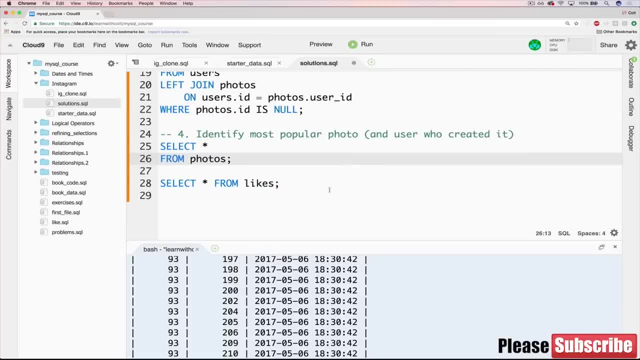 So what we want to work with is the photo ID. We don't care about who is doing the liking, We care about, you know, matching the photos with the likes that correspond to them. So that's going to be a join and it will just be an inner join. 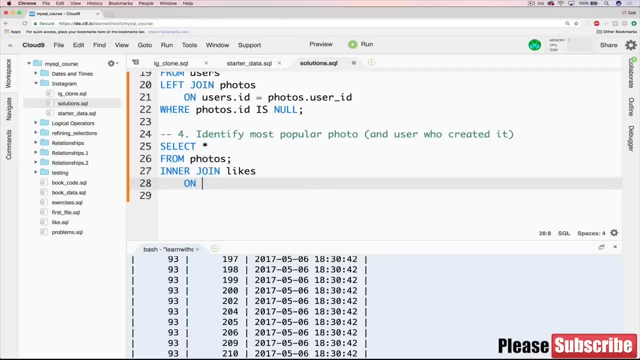 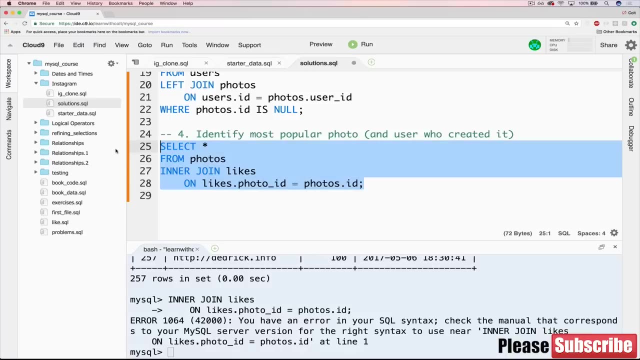 Likes on and we'll do where likes dot. photo ID equals photos dot ID. So this is going to be, you know, a big table here. Oh, what's my error here? Extra semicolon- Try that again. I'll take a moment. 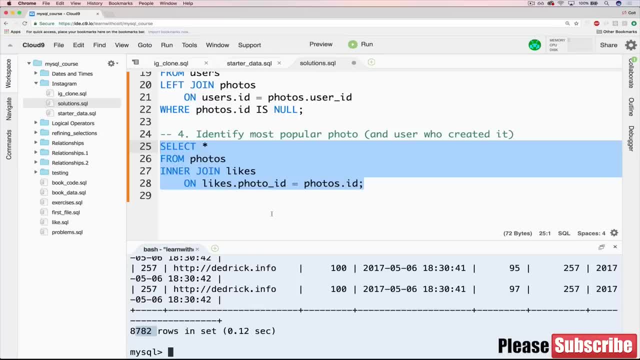 We've got, you know, eight thousand seven hundred eighty two rows, but just like we did with likes, but this time the rows are significantly larger- We have a bunch of data. We don't need most of that. So, rather than just selecting star, which gives us too much information, 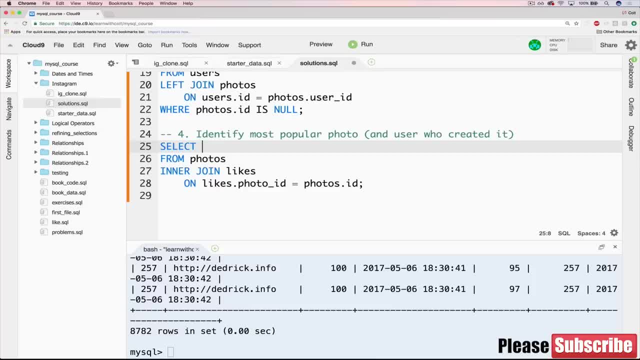 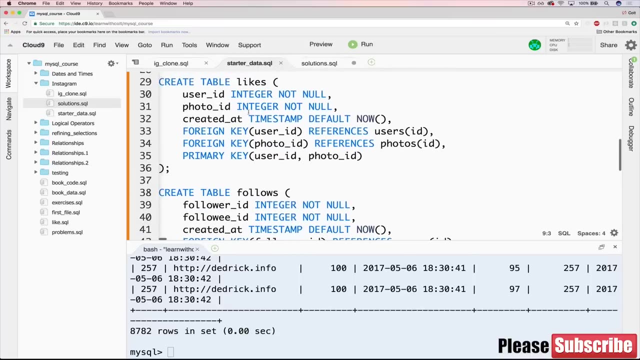 let's whittle it down, Let's call it and we'll just do. Let's see Photos dot ID and photos dot image URL comma. And then what do we have on the likes table? If you remember to go over to our schema here, likes is very simple. 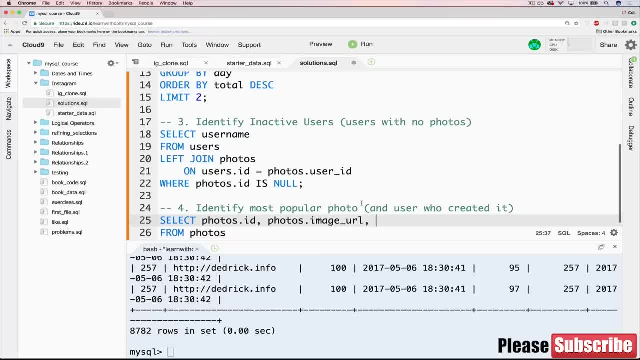 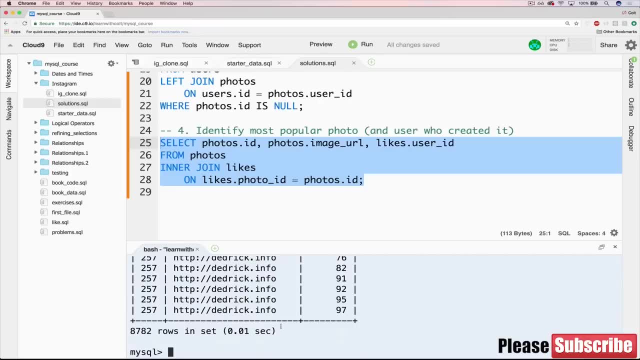 We just have our user ID and our photo ID, So we'll just do what we can do both. Let's just do likes dot user ID to start And you can see All right. So this is all You know on our last photo with ID. 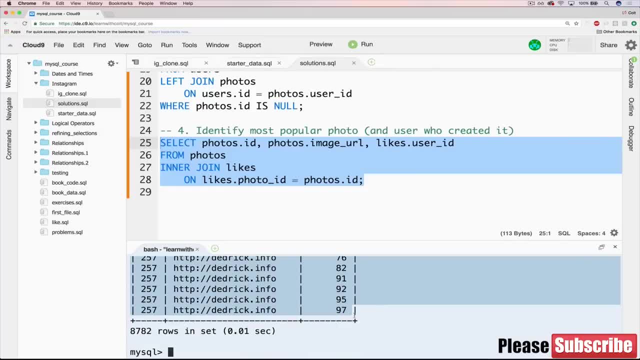 of two hundred fifty seven. all of these are likes for that photo And they are, all you know, by this user or by different users. user ID: three, five, ten, twelve, fourteen, fifteen. We don't need that bit of information. 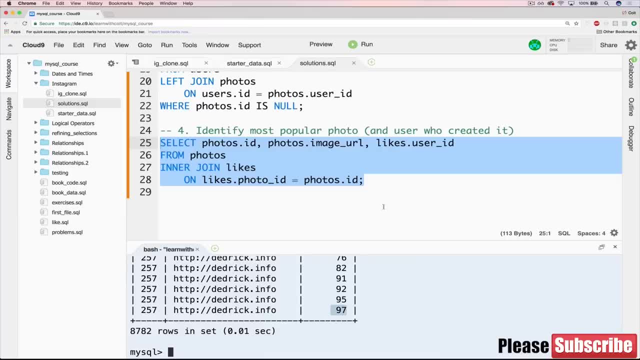 I just want to show you, just so that you can tell we're getting something from the likes table. Now what we want to do is figure out how many each photo has, So we're going to need to do a group by, And before I do that, 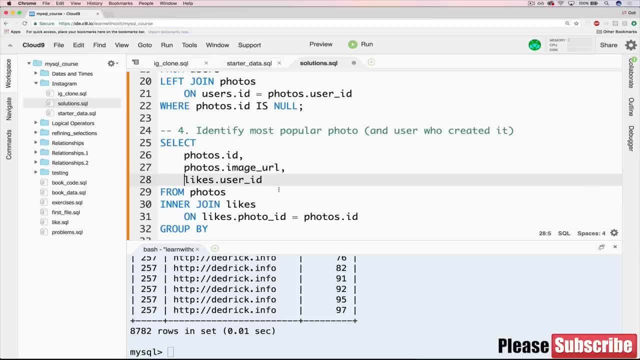 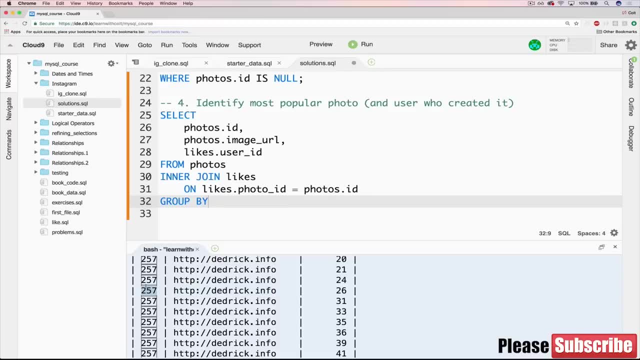 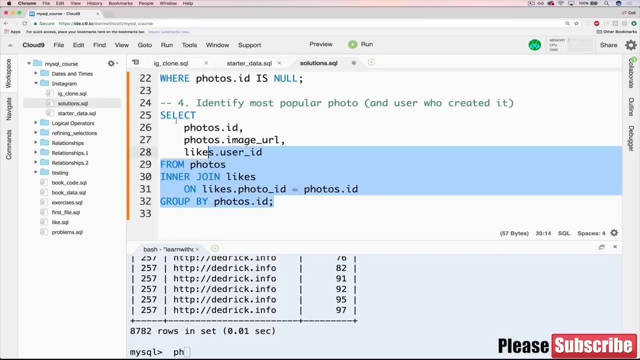 let's just space this out nicely, OK, and we're going to group by. we could do the image URL, but it's much easier just to do it with the integer of the photo ID. So group by photos up here. dot ID. 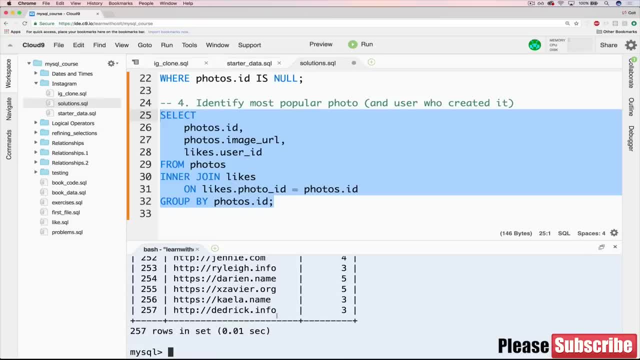 Now, if we do this, we have two hundred and fifty seven rows now, because we only have two hundred and fifty seven photos, And then over here this is still just displaying the first ID of the user who liked that photo. So that's not relevant. 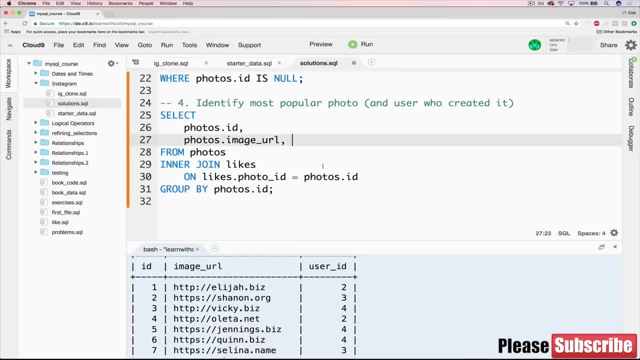 What we actually want to do is display the total number of users who liked it, And that's just a matter of a simple count. Now that we've grouped them by photos, that ID And now you can see over here, you know we've got photos that vary. 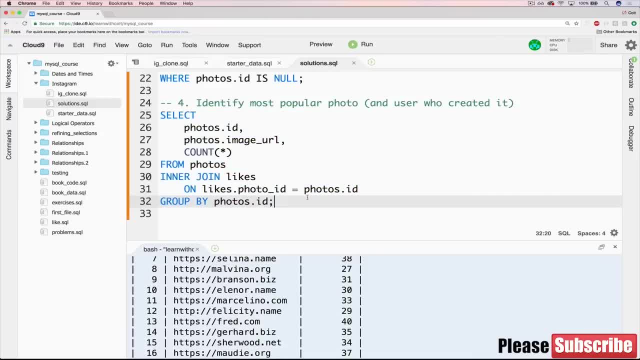 Some of them have a bunch of like, some of them not so many. Now all we want to do is find the number one we could use: maximum or max. I'm just going to do a limit one. for that to work, We need to do an order by. 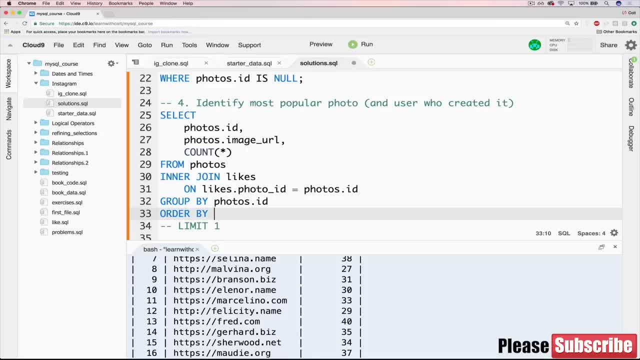 So let's actually start with the order by, And we want to order by count, So I'll give it an alias. I'll call it total: order by total And by default, that will be ascending, which is not what we want. 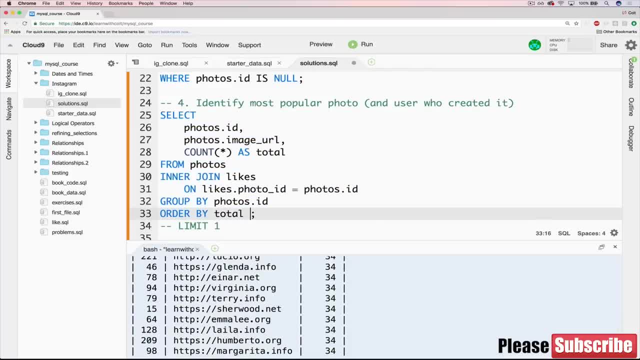 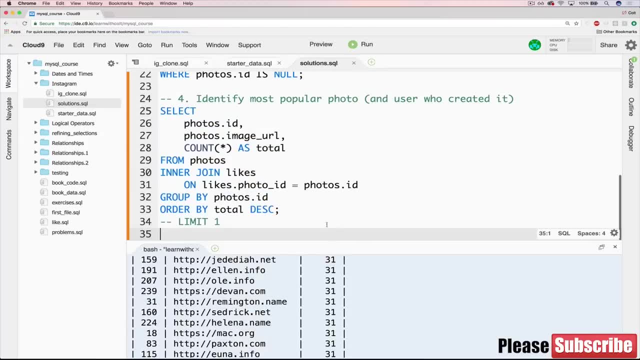 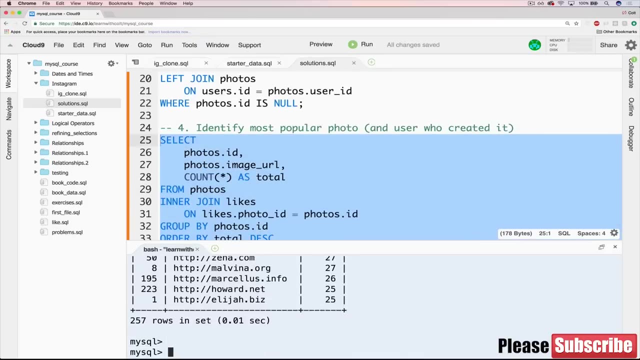 Right, We want the opposite. We're getting there, Okay, Closer. Then, finally, what we want to do is limit it to one and move our semicolon. Okay, So that gives us the name or, excuse me, the ID and image URL and the total number. 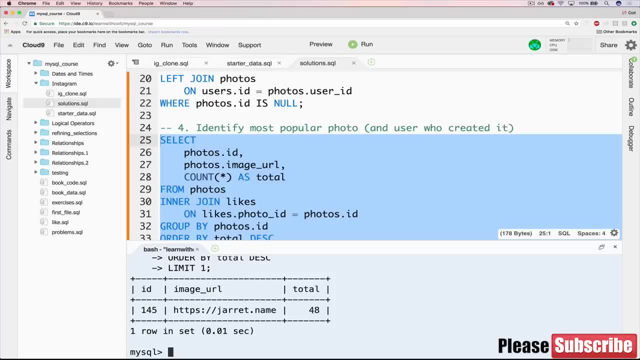 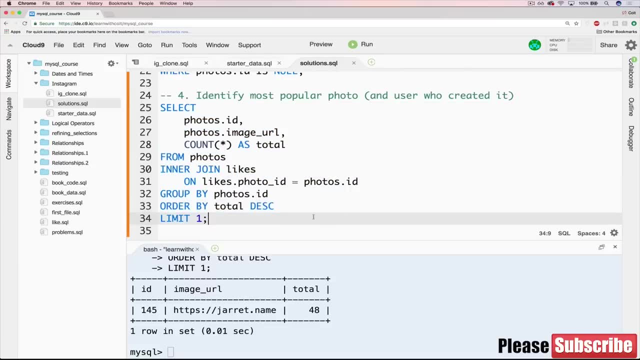 of likes for the photo, the single photo that has the most likes, which for us is 48, and this is the image of the photo. Now we want to figure out who it belongs to, who created it, So we could do a separate query. 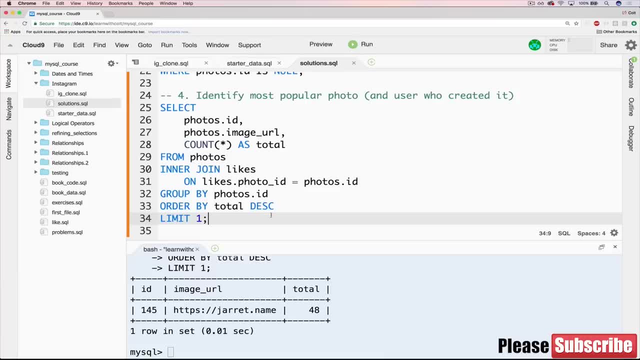 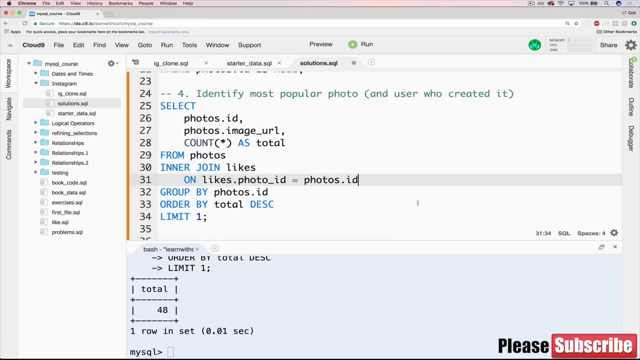 We could even do a sub query if you wanted to, But the easiest way is to do another join, So I'll go ahead and show that join. Basically, all we need to do is get the user information in there as well, And so we're just going to do another inner join, this time on users. 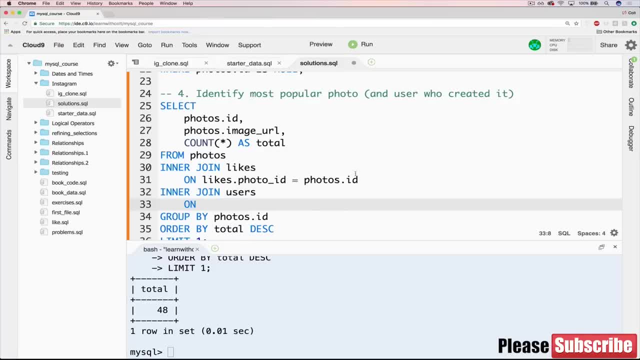 And we're trying to connect it where the- not the like- joint. excuse me, not the likes user ID. that's the ID of the person who liked it. We don't care about That. we want the photos dot. user ID equals user ID. 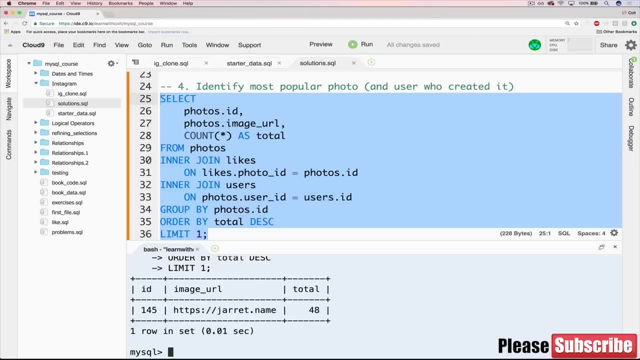 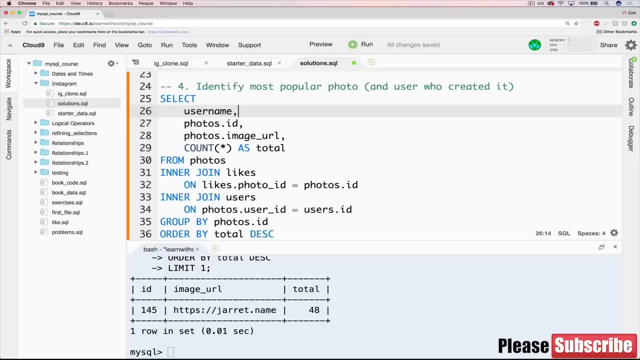 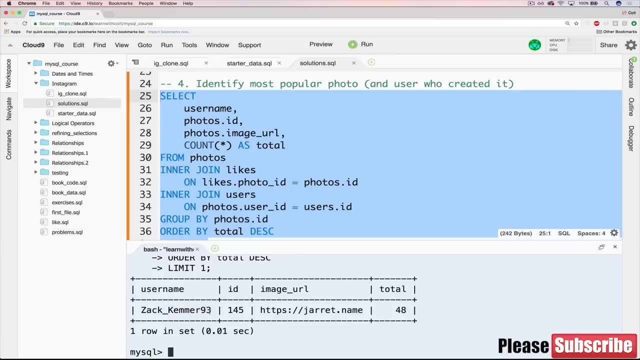 And now you're not going to notice anything right away because we're not displaying it, but we are joining all the user information And all that we really want is user name. So now if we run this, you can see we get Zach Kemmer. 93 with ID of 145 is a person who is responsible. 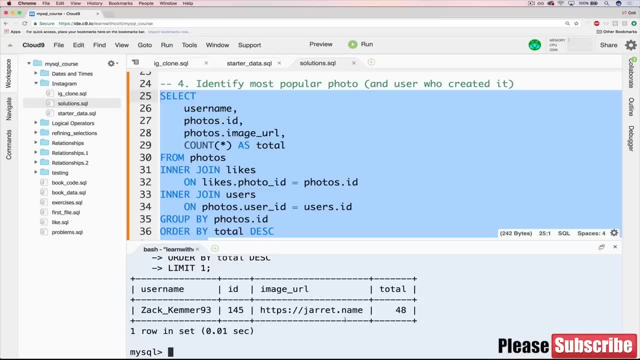 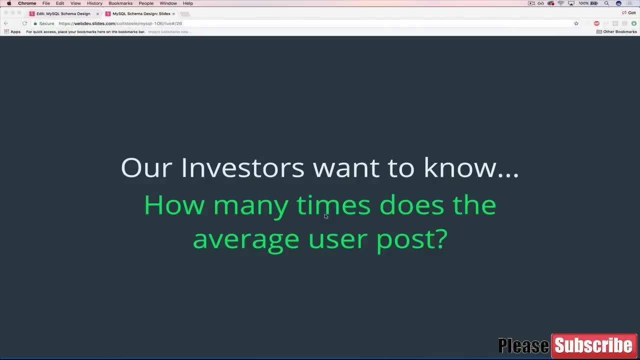 for our most popular photo of all time. This photo, Jarrett name, is our URL, with a total of 48 likes. All right, Next up here. this one will be nice and short. All we're trying to figure out is how many times does the average user post? 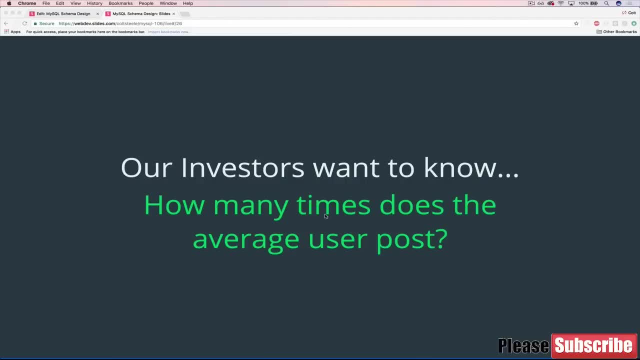 So we have a board or our investors want to know basically what our engagement is like, just in general, for every user, any user. how many times can we assume they've posted? So this is just across the board And really all we need to do is take the 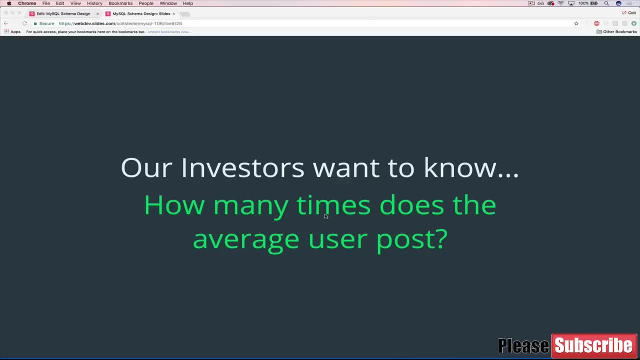 total number of posts, photos and divide it by the total number of users. And you could do that separately in different lines, or you could do a big joint statement between users and photos and then use average and calculate average. But you could just do it using sub queries, which is what I'm going to do. 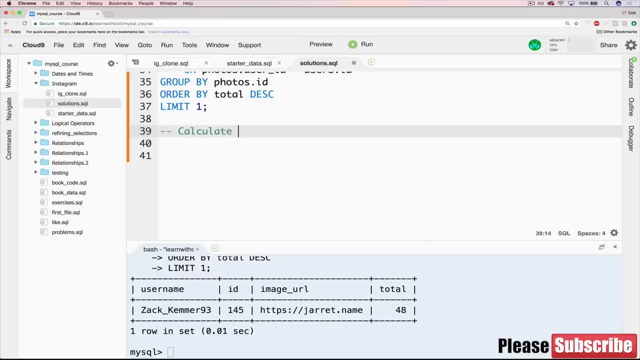 So something a little different. So we'll just do calculate average number of photos per user. So what we're looking for Is total number of photos divided by total number of users And the first part. well, each of those parts individually. we know how to do. 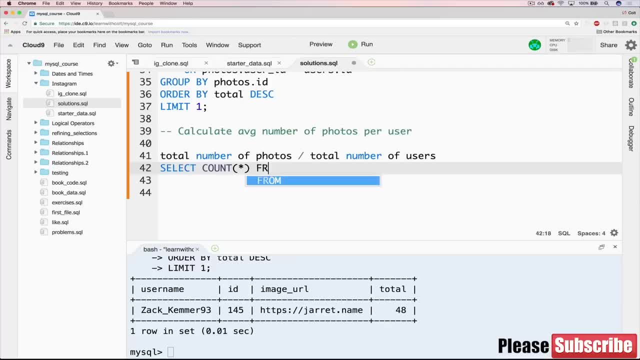 We can just do a select count Star from photos And that will give us the total number of photos. If I had a semicolon, Two hundred fifty seven. And then for users, you just need to change that to be users. Select count from users. 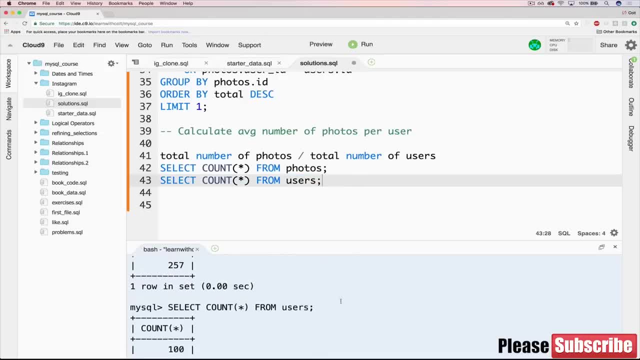 And we get one hundred. Now, if you're good at mental math, even if you're not, it's easy to figure out our average in your head. but of course we're trying to do this dynamically so that if we have X, you know ten thousand more users tomorrow. this still applies. 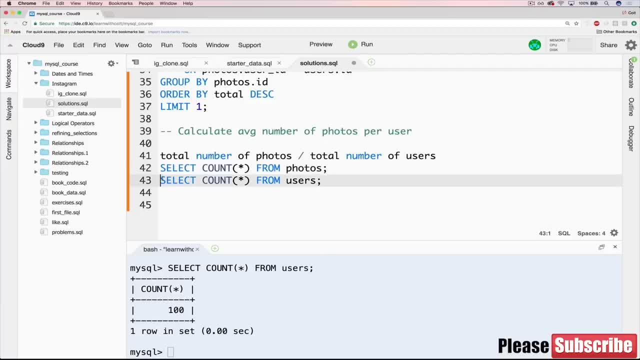 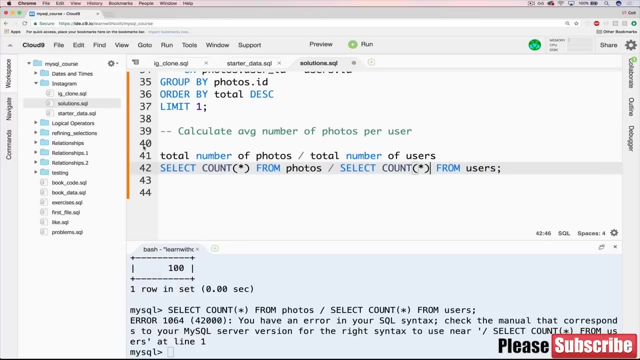 So using sub queries, basically, what I can do is divide these two, So I can't just do this. I'll get a syntax error. What we need to do, like we've seen before with sub queries, is add parentheses, These two things. 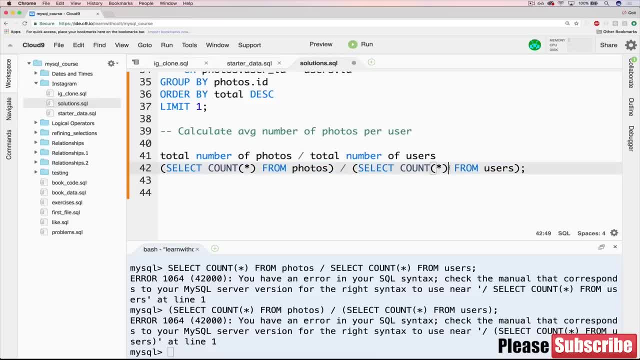 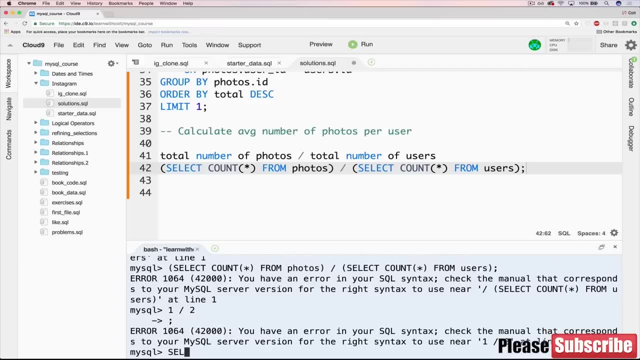 OK, but even that won't be enough. What are we missing? Well, it's just like we can't just say five plus five, We can't just do one divided by two. We have to say: select one divided by two in order to get anything. 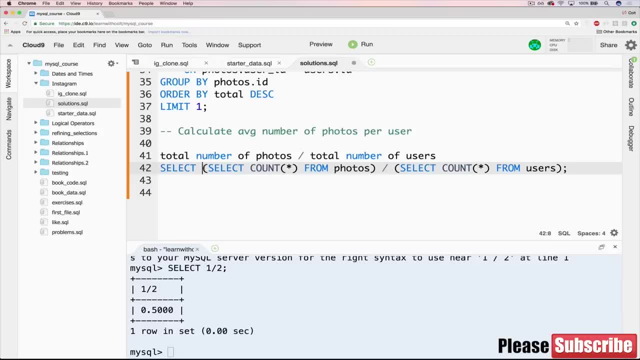 So we need an extra select up here. Yeah, it's kind of a mess. You know we could do this on separate lines, Maybe. I'm not actually sure how to best format this, because it's kind of a weird query, but maybe something. 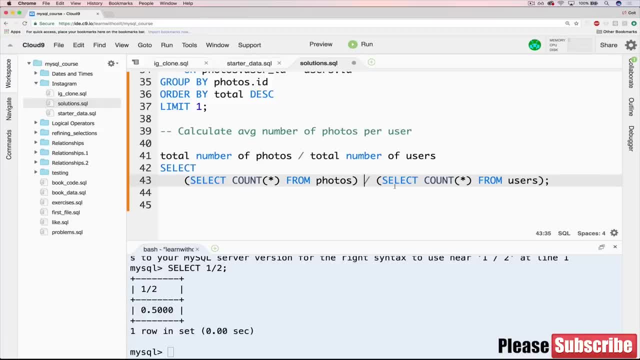 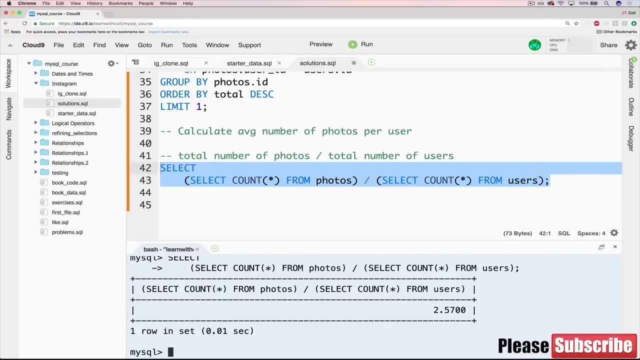 Like this: Well, we can leave it at that for now. I'll get rid of it. I'll comment that out now. If we run this Well, we get this massive line here, but two point five seven. So every user has two point five. on average, every user has two point five. 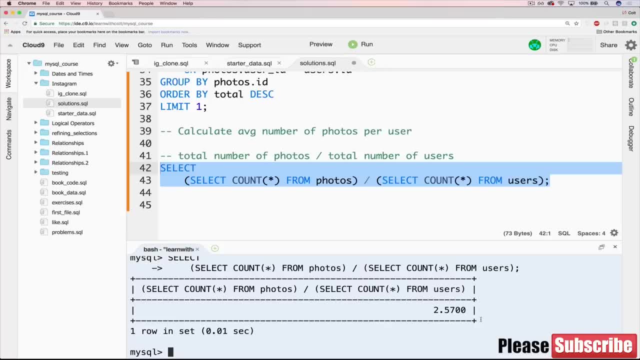 seven posts. that's thrown off significantly for a couple of reasons we'll see later. There are bots and users who just don't post anything, And if we tried to get rid of these bots our average would change. So we'll get there in a moment. 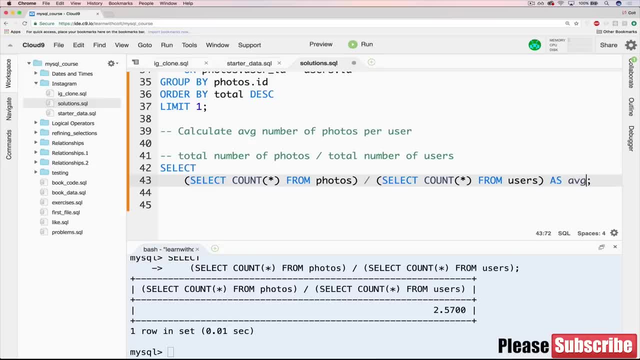 What we could do is just add in simple alias. We'll just call it as average ABG. OK, and there we go. So that's the answer to that one. If you came up with another way, feel free to share it. 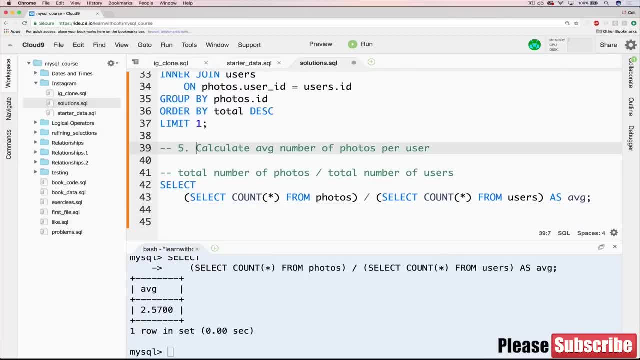 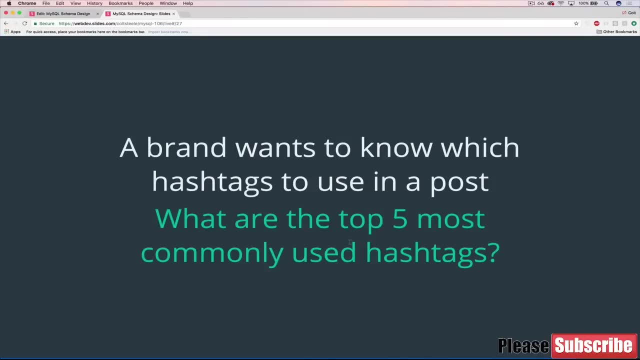 And we'll talk about it in the comments. All right, Moving on. OK, so next up, you know, suppose, getting the brains of our Instagram clone application employees, And we make money by having sponsored content, by having advertisers post things on our app. 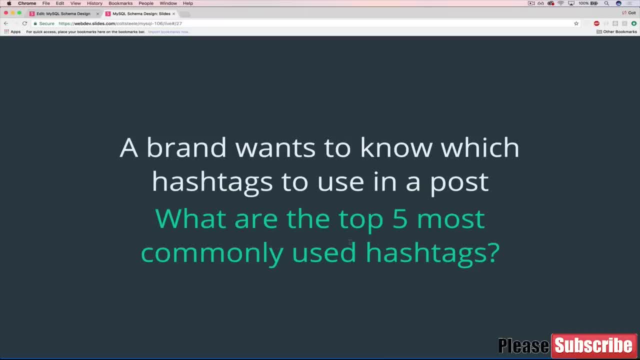 And they want to know what hashtags they should use which are most popular at any given point. So what we want to do is just find the five most commonly used hashtags so we can tell our advertisers these are the hashtags you should use on your own stuff. 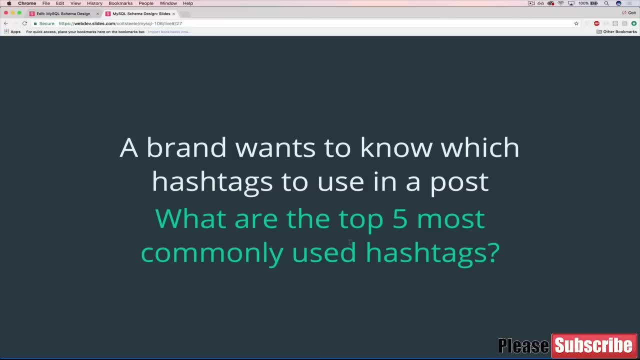 because they're trending right now to what people are looking for. So to do it, it's pretty straightforward. We have a single join. We're basically going to connect hashtags or tags with photo tags. Remember, we have those two tables. The one table is just the name of the tag. 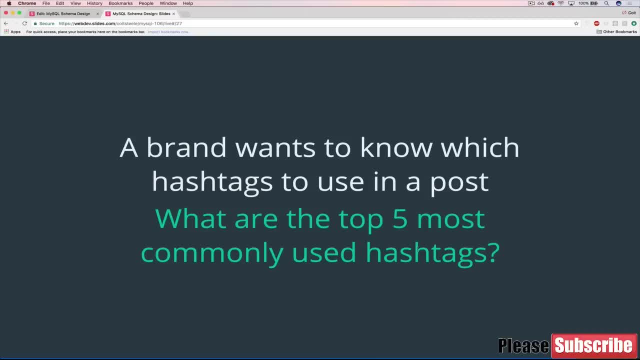 and the other table is every time the tag is used and applied to a photo. So we want to count. Basically we want to group all of those photo tags together, count them, But then we want to find the associated name of the tag. 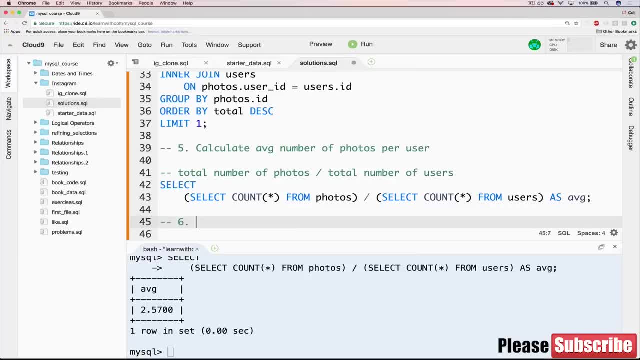 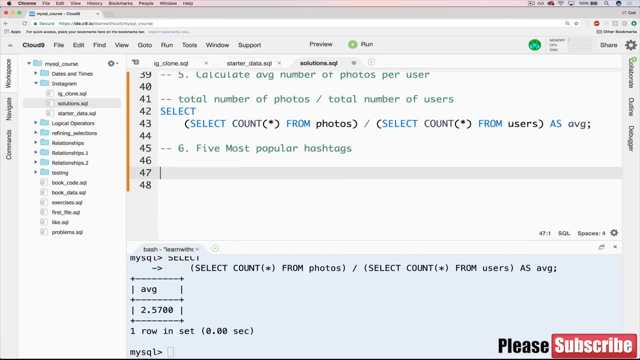 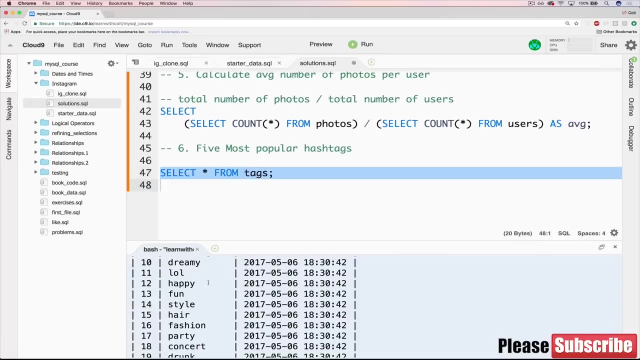 So let's start that We'll do six most popular hashtags. Five most popular hashtags. So if we start with just selecting star from tags, as we've seen before, it's just a list of the hashtags themselves and then an ID, a hashtag name. 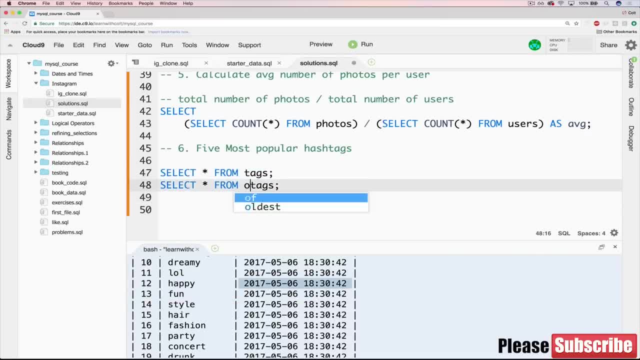 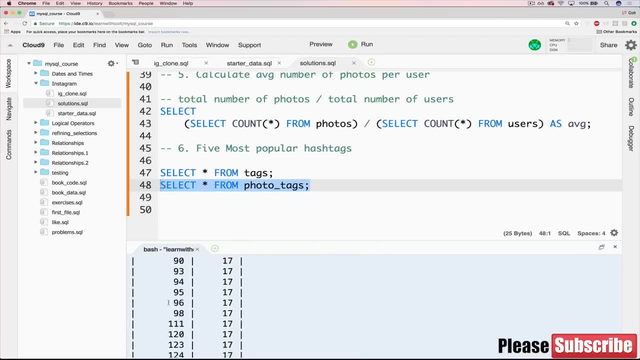 and then created that. But we've also got photo underscore tags and we've got a bunch of those- 500.. And each one is just a hashtag or a tag ID and then a photo ID that it's being applied to See if we can get to the top. 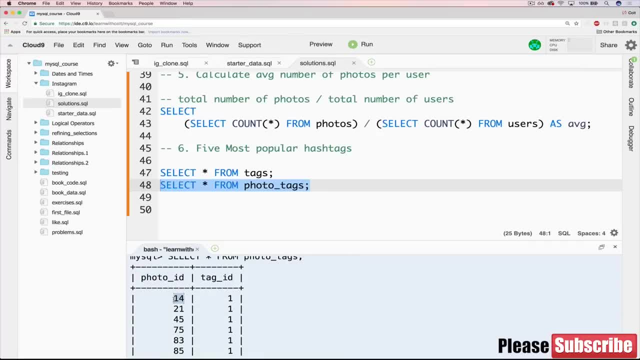 Here, Here we go. So the photo ID, photo ID 14, is being tagged with whatever has tag ID, one which is sunset, So photo 14 has the tag sunset. So what we want to do is we can start, if we wanted, by just focusing on these. 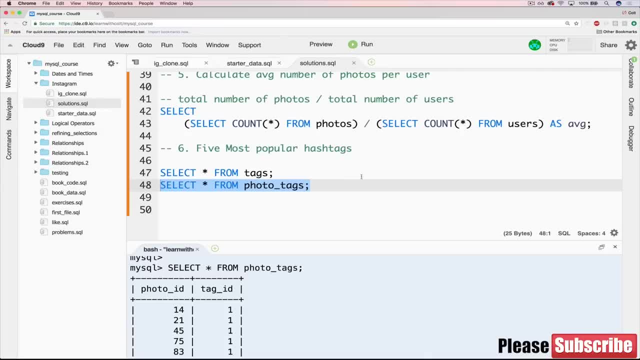 and counting how many times each tag was used. But it makes it a little easier to follow if we join tags. So we have a name of the tag as well. So we'll do that. We'll do select star from photo tags And then we'll do join tags. 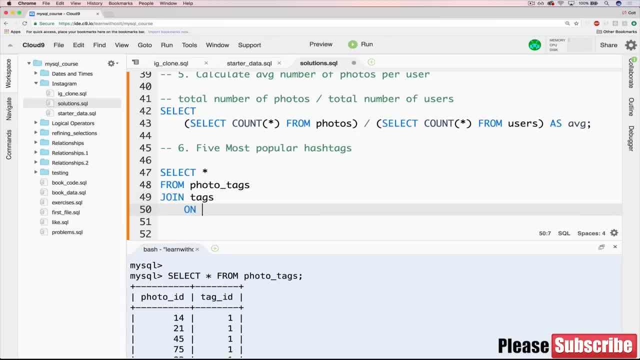 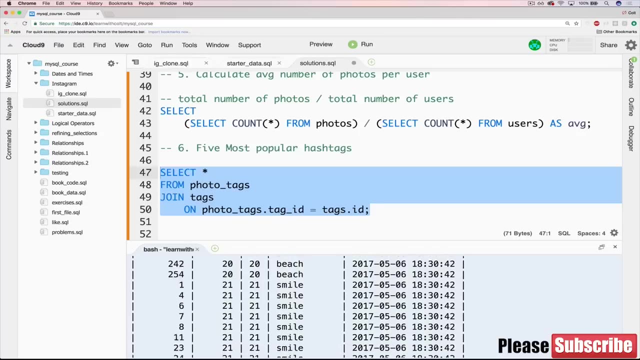 Get rid of the other stuff here. on photo tags, dot tag ID, which is this, where this tag ID equals tags ID. So now what we see? there's a lot of stuff: 500 rows. If we go up to the top we can see they're already being grouped. 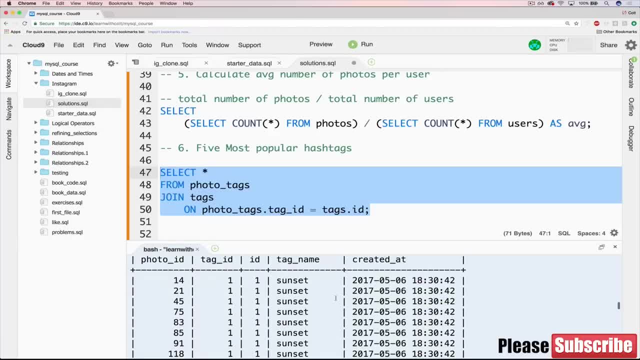 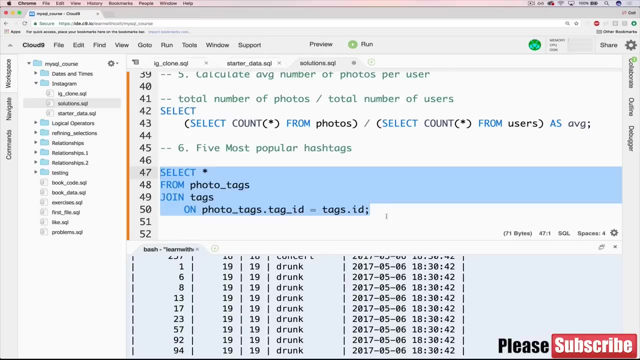 Roughly, Not exactly, but they're being grouped roughly by the tag name. So we've got: 14 was tagged with sunset, 21 was tagged with sunset, 45 was tagged with sunset, and so on. So then what we want to do is basically collapse them using group by. 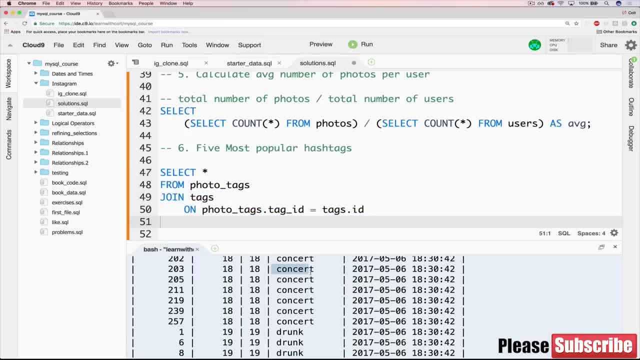 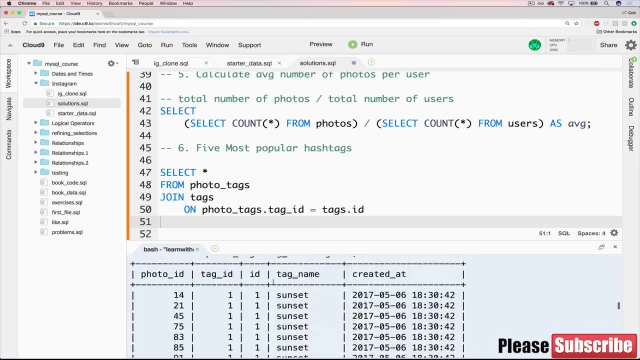 And we could use the tag name to collapse them. But we could also use the tag ID, which is easier because it's just a simple integer rather than having to work with strings and text. So we'll do the tag ID. So that's group by tags ID. 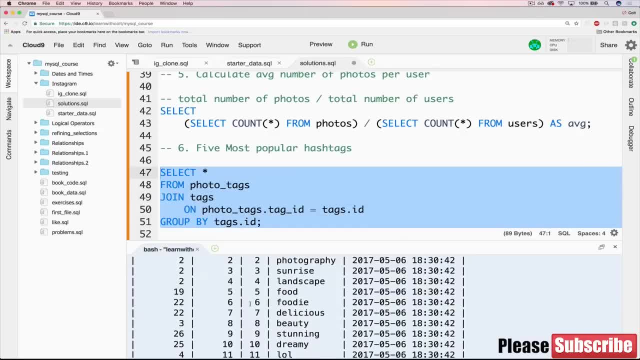 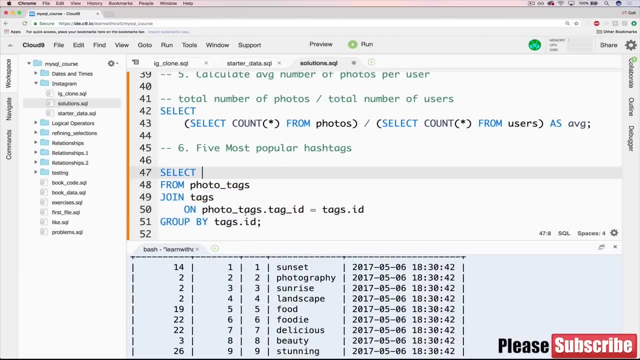 Now we do this, We're getting closer. Now we only have 21 because I've been grouped together. Then, finally, rather than selecting star, let's select the tag Tags: dot. tag name, comma. Do these on separate lines. We want the count. 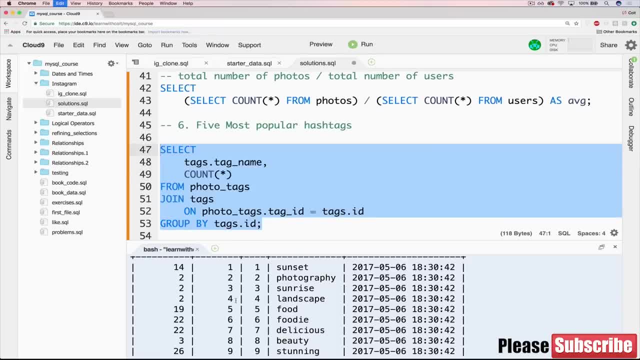 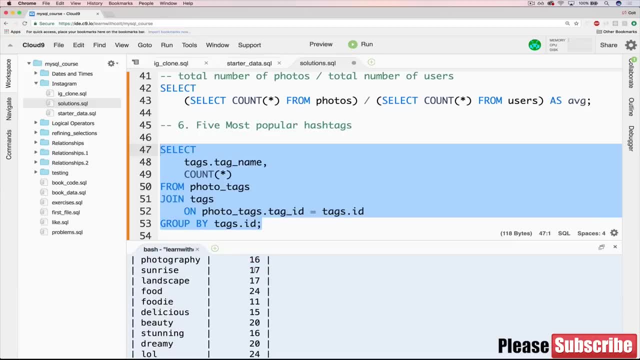 Star: OK, so we can see things like: sunset was used 19 times, photography 16 times, sunrise 17 times. then we'll go and give this an alias as well. Just call it as what's a good one: total, OK. next up, we want to find the maximum. so you could use max, but would be better. 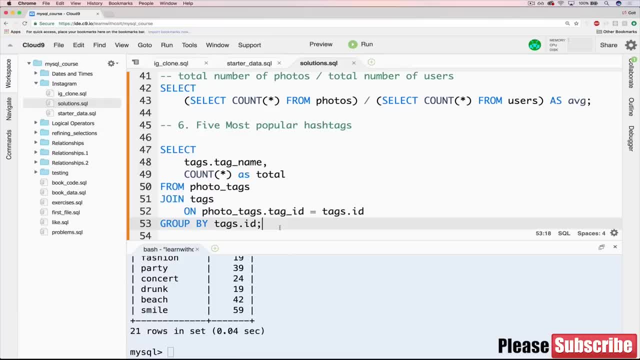 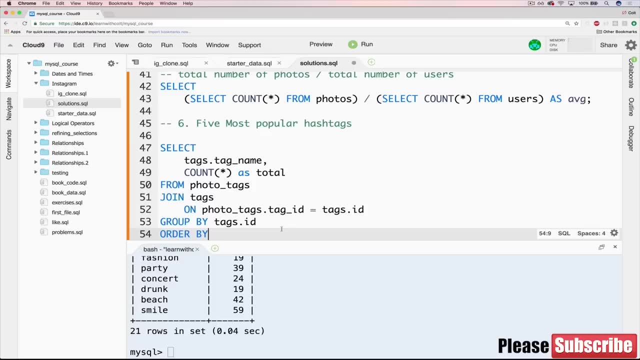 And what I'm going to do is just use order by and then limit because we want the five most popular. So actually you couldn't use max because we want five, So we'll do order by. what are we ordering by? this count here, which we called total, 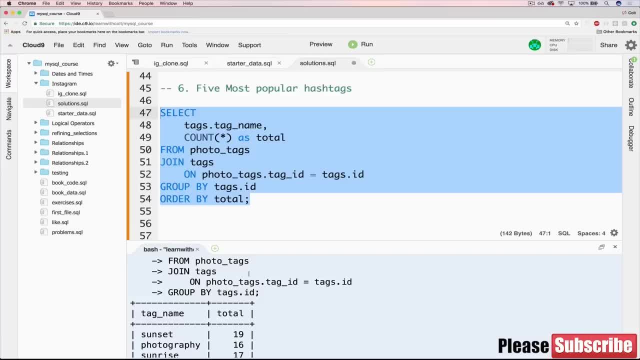 order by total, and if we do that it will be in ascending order. So we want to change that, And then we want to limit it to five, and that should do the trick. And there we go. We see that the top five tags right now. 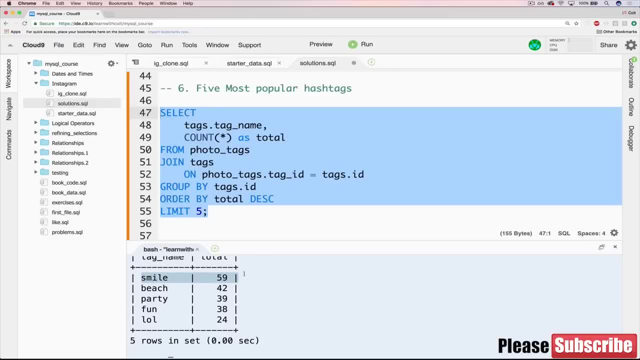 Number one by far is smile. Apparently it's very popular and we've got beach at 42 party Thirty nine fun and LOL And I know for a smile and I kind of engineered to be there because when I was making the data I wanted some hashtags that could be used. 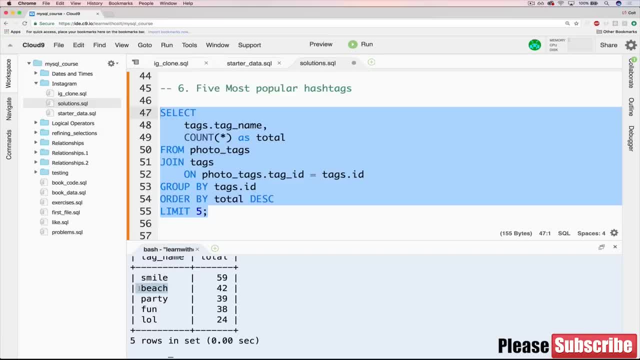 in multiple contexts and things like beach could be used in a landscape photography shot alongside sunrise or sunset or landscape, but it could also be used in a model photography shot alongside model or beautiful. It could be used in a party alongside a party hashtag if it was a beach party. Smile can be used in a lot of. 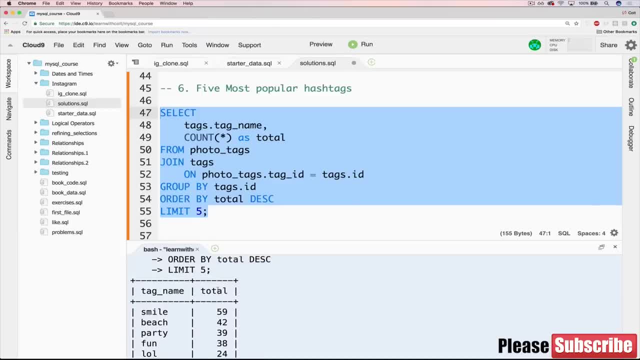 ways. So can party. So, anyways, I tried to come up with certain tags that could be used in different ways, And there we go. Those are our top five hashtags at the moment. Next up, you guessed it something else. All right, next problem here: This is a little different. So, as I mentioned, 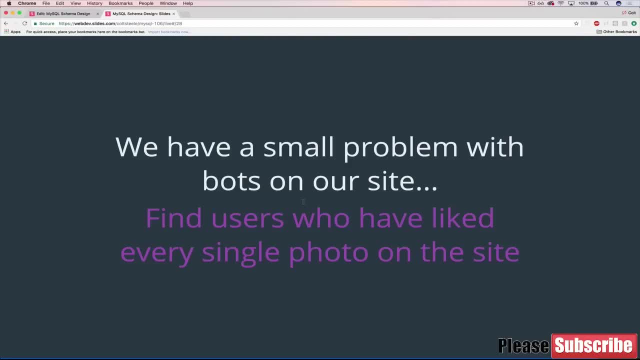 earlier. a real problem on Instagram are bots- bot accounts that basically exist to go around and like a bunch of stuff or to comment on people's things but not create their own content. They're not real people. Oftentimes they're commenting the exact same thing Or like if I post a photo. 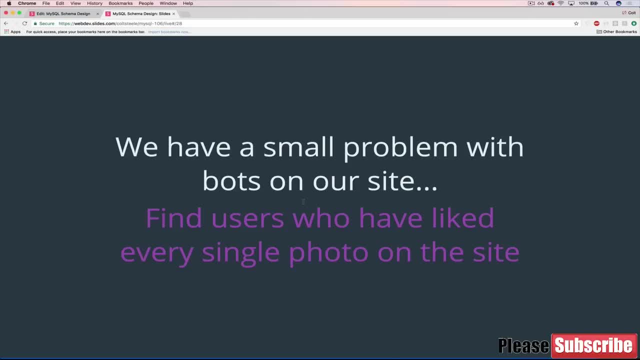 I'll notice I get like 10 likes immediately, like the next second And usually there's not 10 people who are happening to you know to like it immediately. There's some sort of program that's happening behind the scenes where it's looking for new posts and liking them immediately. So in our hypothetical Instagram, 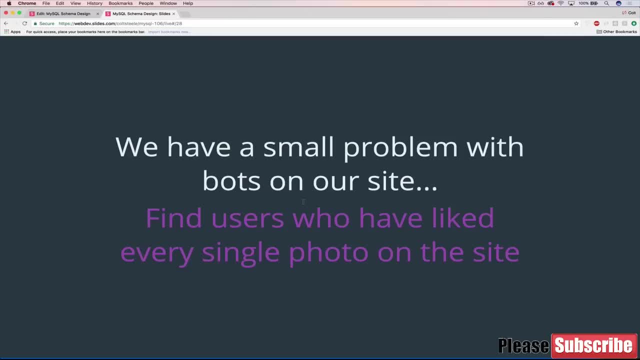 clone. we have the same problem. So what we want to do is just find all the users who we think could be bots. They're users who have never excuse me. they're users who have liked every single photo on the site. So if we have 257 photos, they've liked all of them. If we have 800 photos, 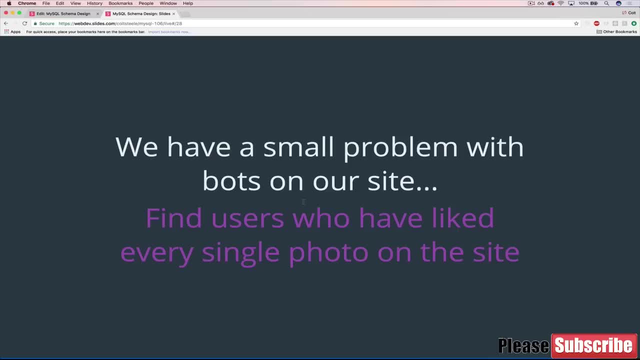 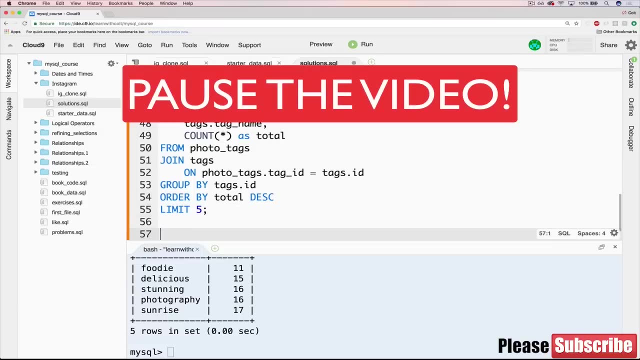 they've liked all of them, And I'm going to show you a way of doing it that actually uses something we haven't seen yet, something new. So go ahead and give it your own shot, And then we'll have a solution. Okay, so the first thing we want to do- we know it's going to be a join between users and 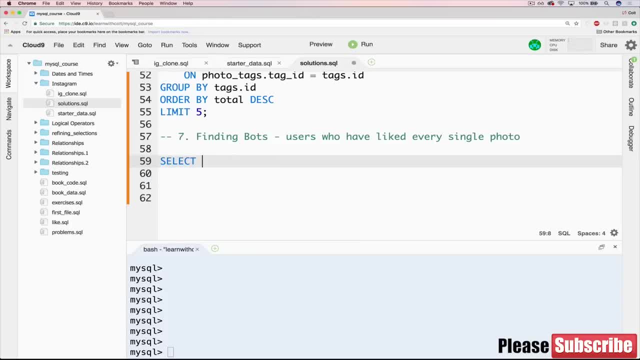 likes. So we can start with a let's do select star from users And we'll do an inner join likes. And the reason we know it's an inner join because we don't care about users who don't have any corresponding likes or likes that don't have a corresponding user. So it's. 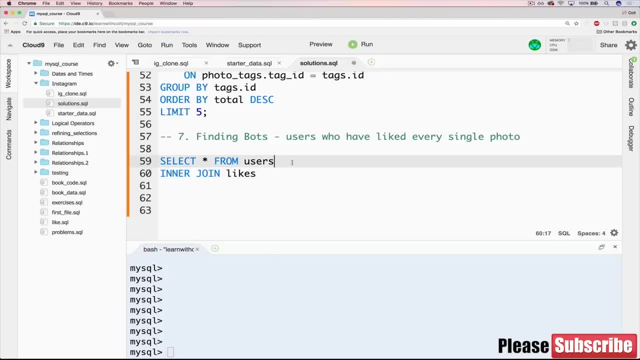 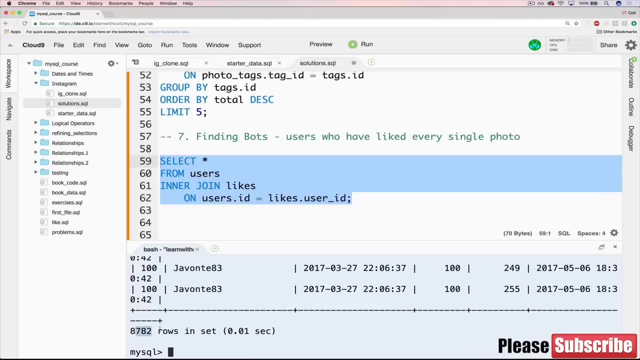 exist. So we want the inner join, we want the overlap only. So select star from users. inner join likes on usersid equals likesuserid And if we start with that, takes a moment. you've got remember 8782 likes And now what we want to do is group them based off of the user. 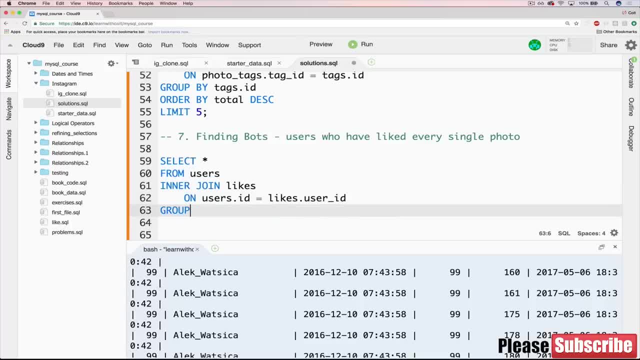 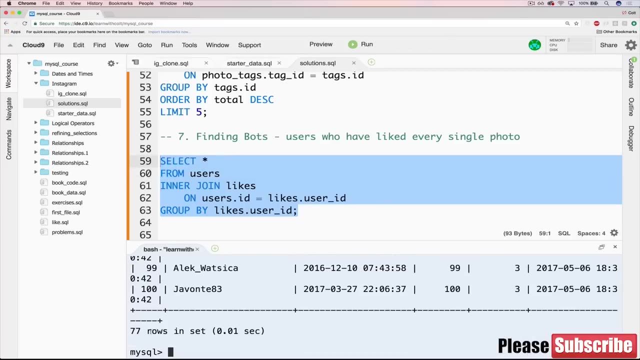 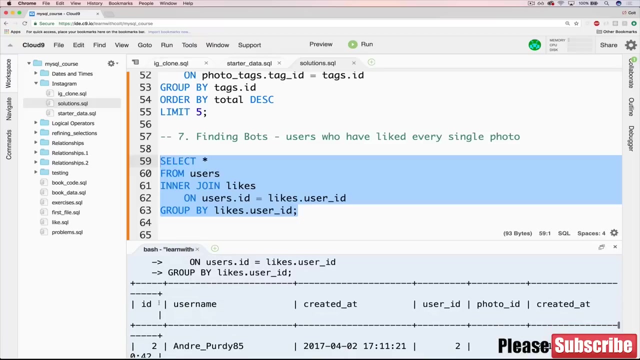 who did the liking. So we'll have a group by and we have a bunch of likes, choices of how we group them. We could do usersid Or we can do likesuserid. We'll save, Okay. so now we have 77 rows here And we can see. you know, there's a bunch of information. we've got the. 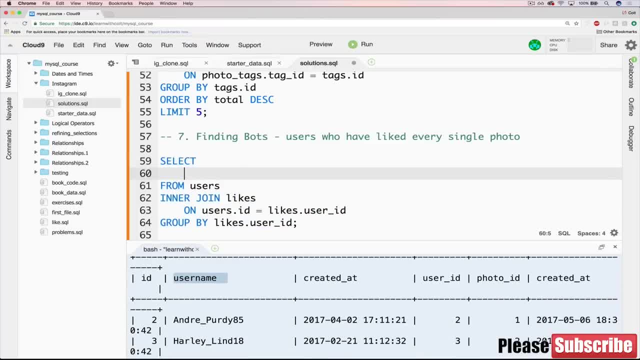 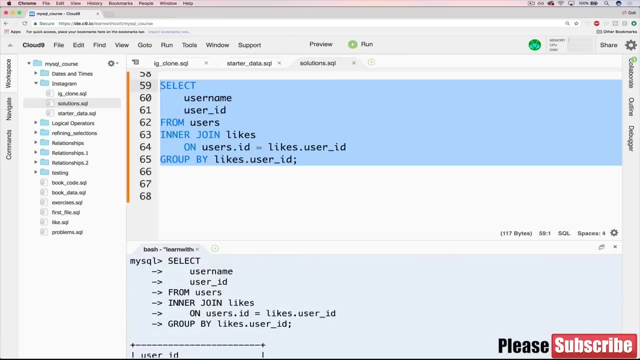 username we don't need created at. So let's slim this down a bit. Let's do select username, user ID, And we'll just keep it at that. Okay, so these are all the users who have liked anything at all. 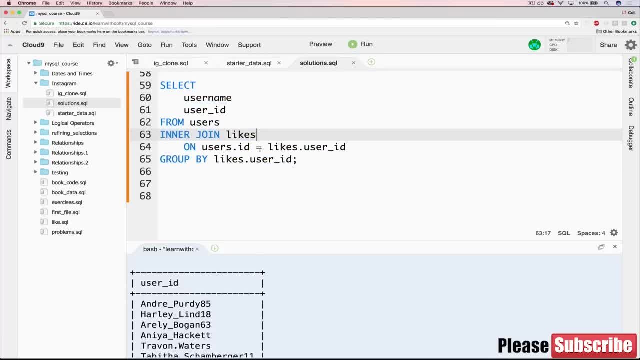 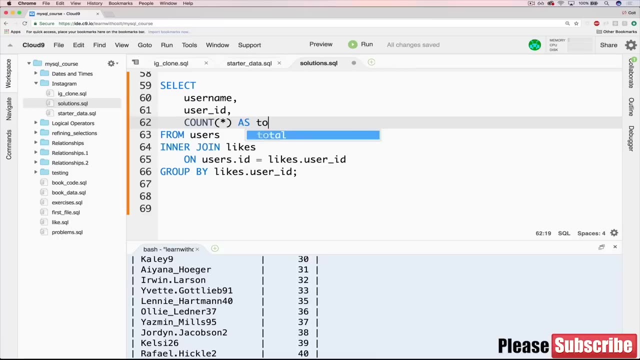 We're grouping them right, So they're grouped by user ID. I'm missing a comma. That's what's going on Now. what we want to do is figure out how many. So that's just a matter of using count star, which you should feel pretty good about Now. we'll give it an alias right now. 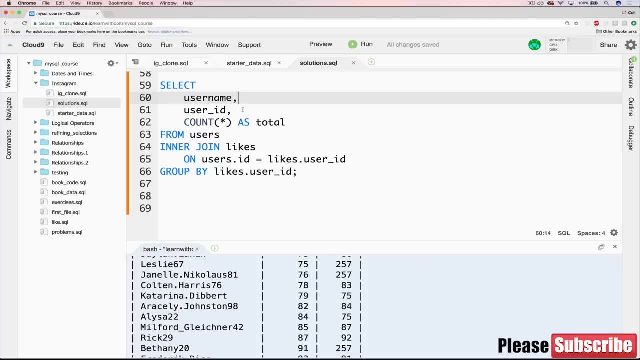 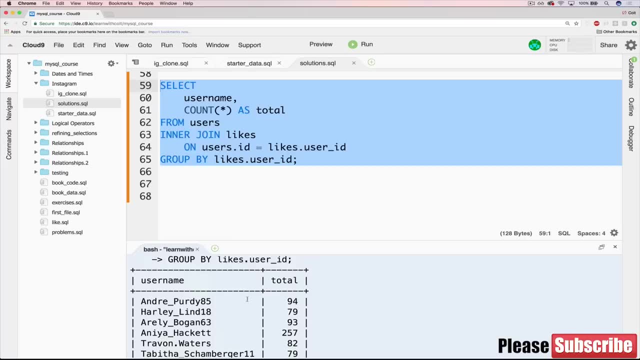 Okay, and we can get rid of user ID as well And just do username. Okay, so we can see that. you know we have Andre Purdy. 85 has 94 likes. Let's give this actually num likes, But the question was not just to figure out who has. 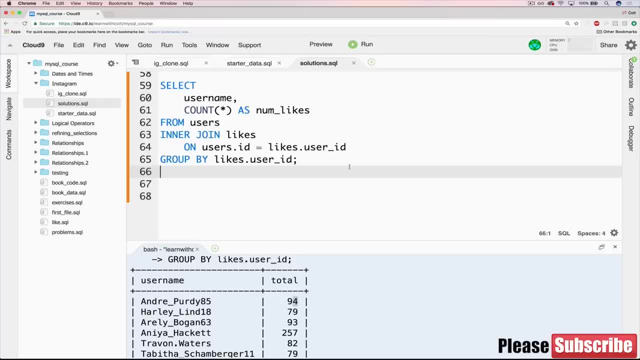 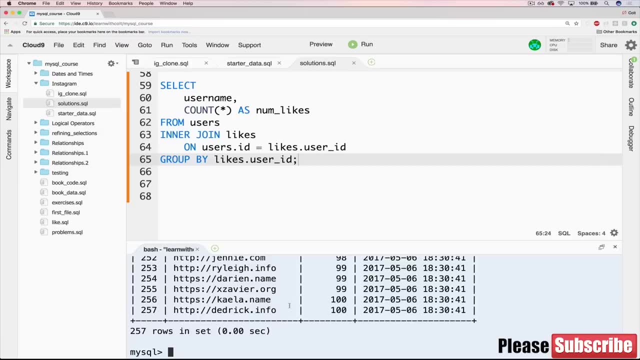 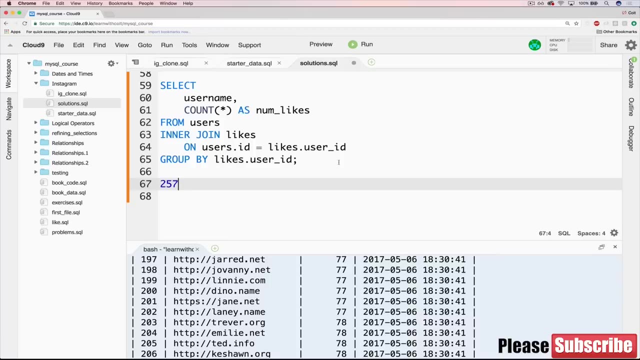 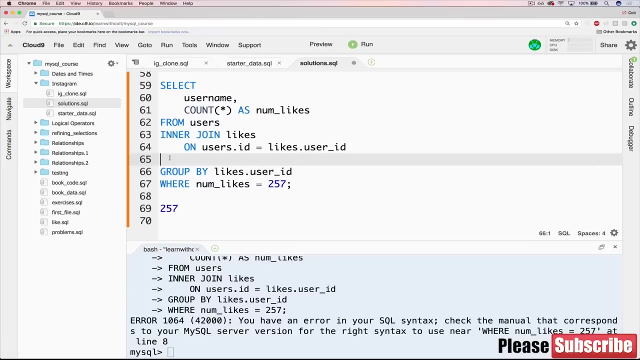 the most, but to figure out the people who have liked every single photo And you know if you don't remember how many. we have 257. But we're not talking about cheating And we could cheat if we wanted to check exactly for 257. It's not too bad. But you might think you could just do like a where where num likes equals 257. But that won't actually work And that's because where clauses actually go before the group, by telling it what the data you'd like to select to group versus what you'd like to select from the group by 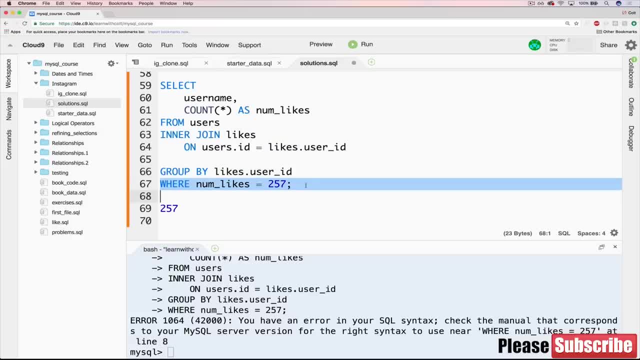 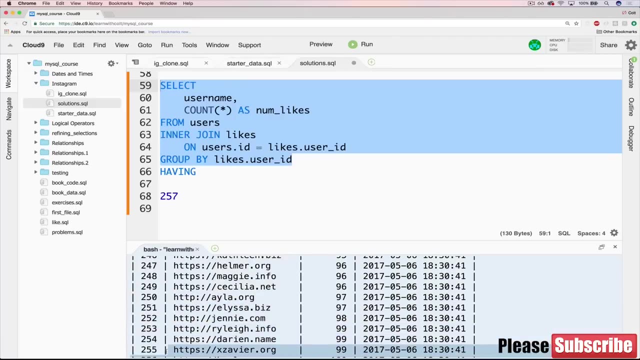 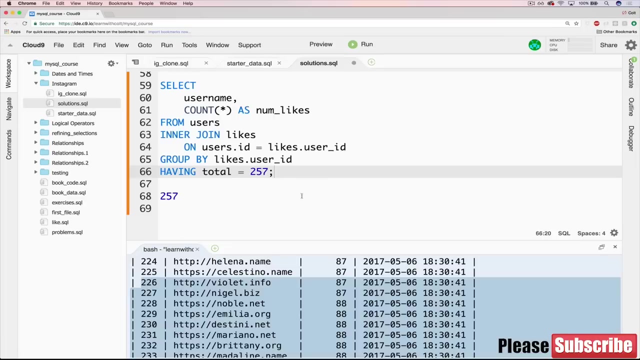 Okay, so now we have 257. So what we're going to do is we're going to copy the data we've just copied into our group And then we can see that we have a little bit of a difference between the two here. So because the data we got from having and having and other things, we want to filter it out. And the way we can do that is we're going to say having acts like. where will do this? So if we use the group's data, So where doesn't work. we need to use something different, which we haven't seen, which is called having and having acts like where. it's just a different word And what it will do is take our group's data or end result and allow us to filter based off of a clause. So we can say having and we want to say total equals 257. Just like that. So now if we do it- oh, total, I changed it to, oh, I was wrong. So we're going to have some sort of filter here. So if we do a group, then we can. 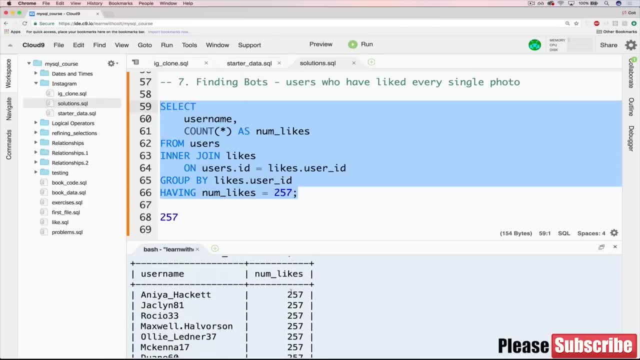 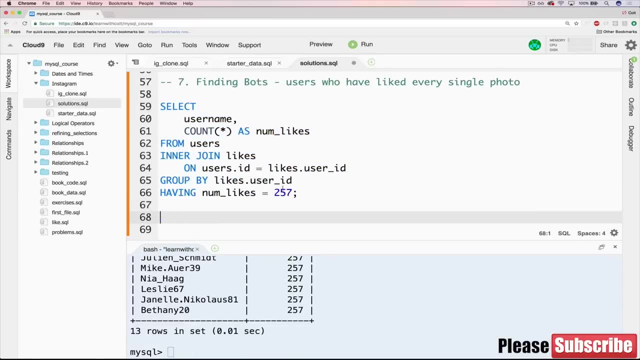 to name, to num likes, but now, if I do it, you can see: okay, these are the people who have liked it 257 times, like every single post. but the problem again is we hard-coded 257, so we could fix that very easily. we want this to be dynamic, however many photos we have, and we can just use a sub. 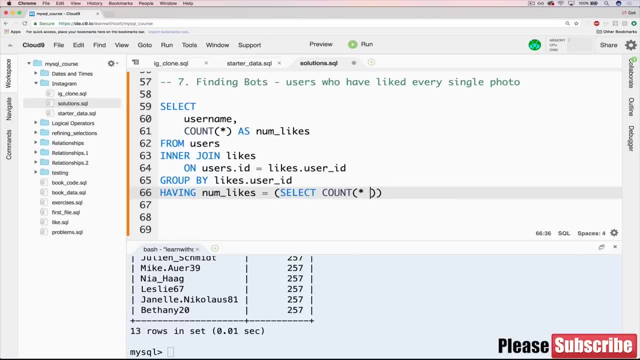 query to select count star from photos. so this will be where the number of things they've liked is equal to the total number of our photos. and there we go. we get the same exact thing, but this time, if I add a thousand photos or remove 10 photos, this will still always be the total number. 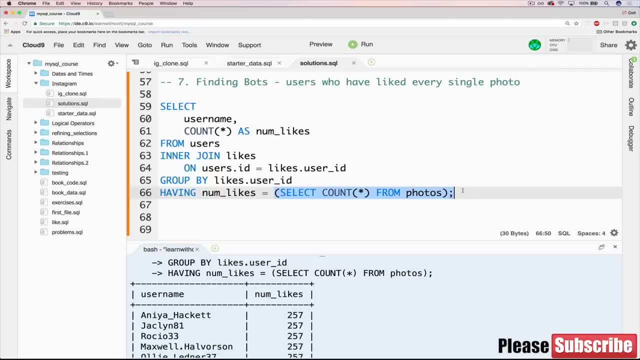 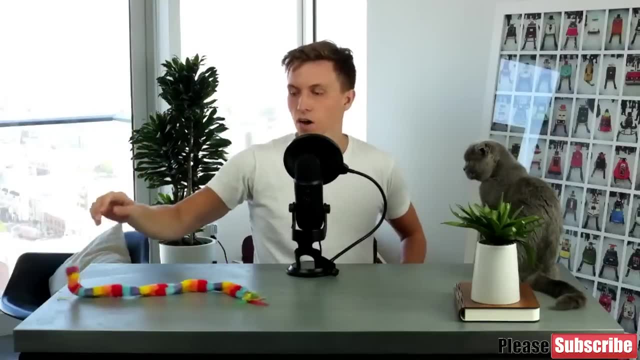 of photos. okay, kind of an ugly query with this sub query here, but if you came up with something different, post it. we'll have a discussion. hey there. so this section is all about node nodejs and the core of it is: how do we take a programming language? 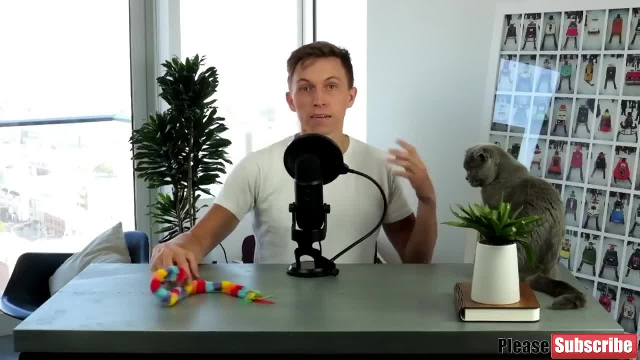 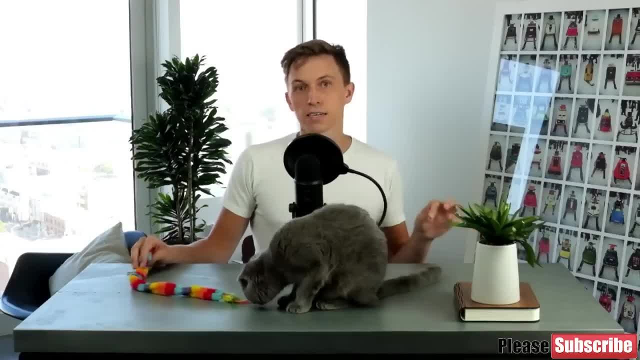 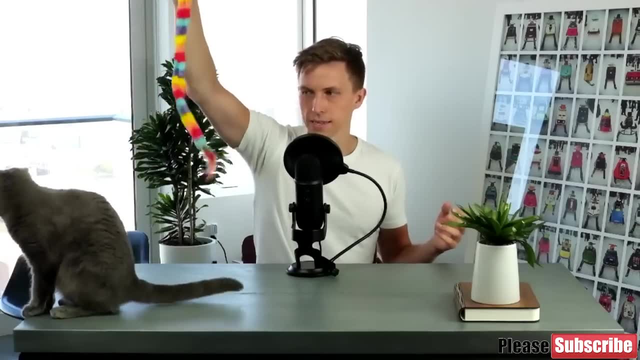 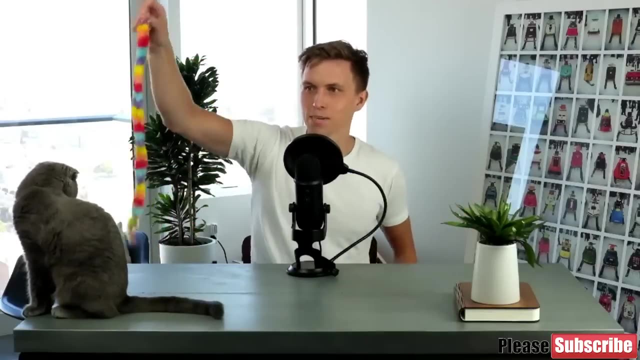 that we can do things like build web applications, and in this section we're not getting to the web app just yet. so for a lot of you I know that building a web app has sort of been like the- whatever you call this thing- the catnip, I guess, or the, the toy that has been dragging you through. 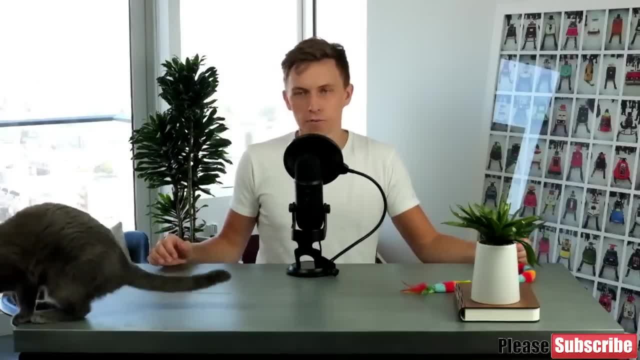 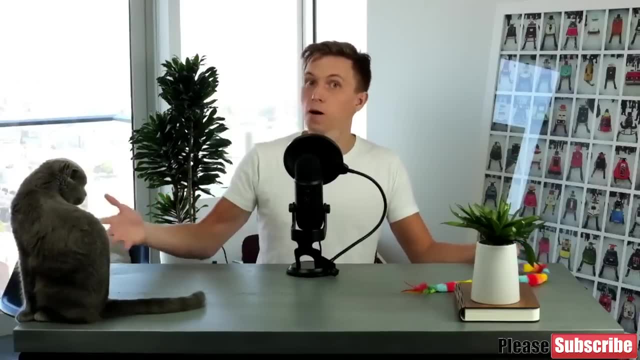 this course, getting you through the more dull part, knowing that you'll see how to make an app at the end. but remember, this is not a web application course. this is a course on my SQL, so it's just a small part. but if that's what it takes, it's the light at the end of the tunnel. well, we're. 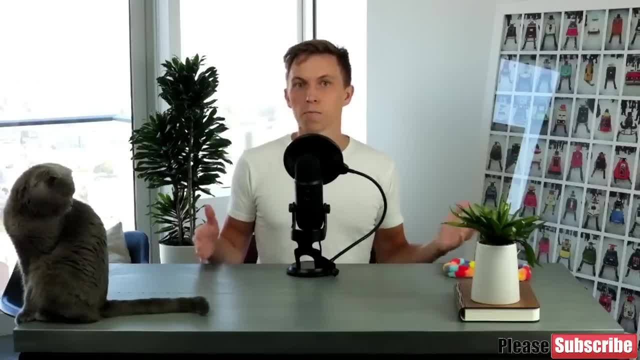 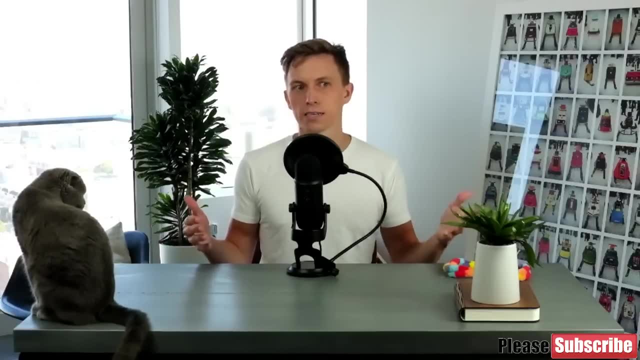 basically through the tunnel now and, like I said in this section, we're not building the web app just yet, but we are seeing how to connect my SQL to another language. in our case it's nodejs, and so what we're gonna do here kind of it's a tricky situation for me because I don't have the luxury. 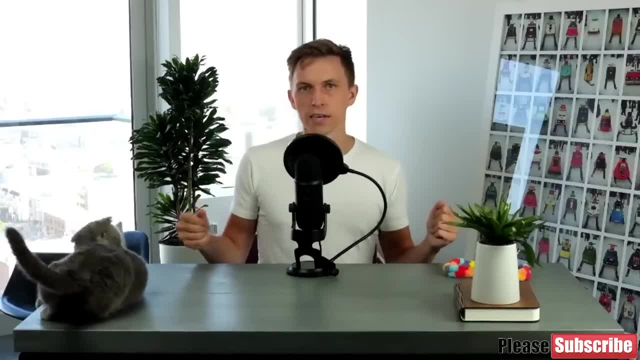 of teaching everybody node and teaching all the people that I know how to use nodejs, and so what we're gonna do here kind of it's a tricky situation for me because I don't have the luxury of teaching everybody node and teaching all the basics that you need. so we're kind of going to do a crash course at the beginning then 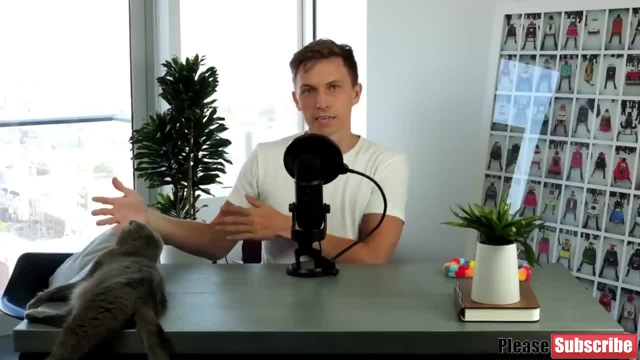 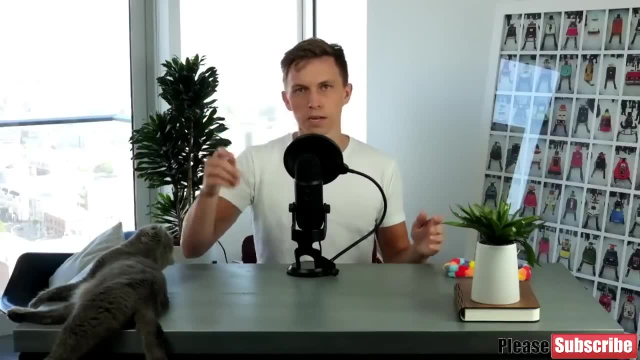 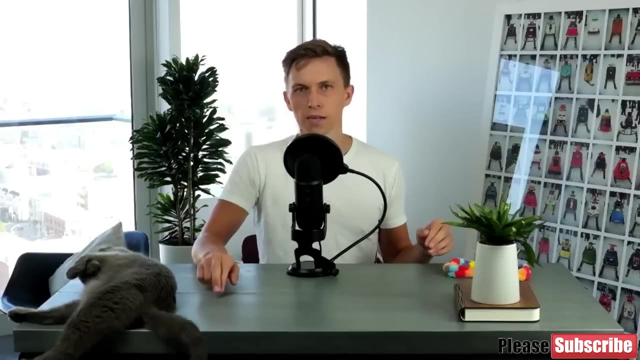 we're going to work with a file of JavaScript and connect it to a MySQL database so that we could do things like randomly generate 500 users and insert all of them with one go. so we can insert, you know, 500 users manually. but how could we make 500 random users every time I run a file? that's 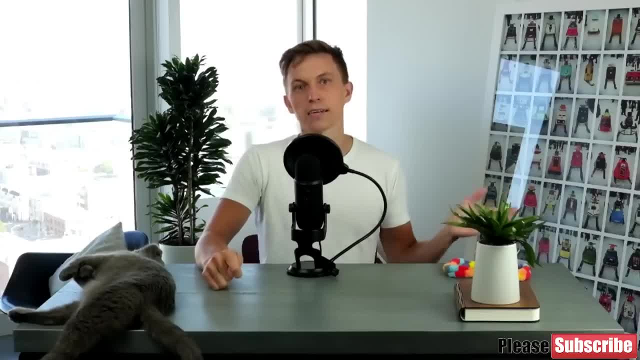 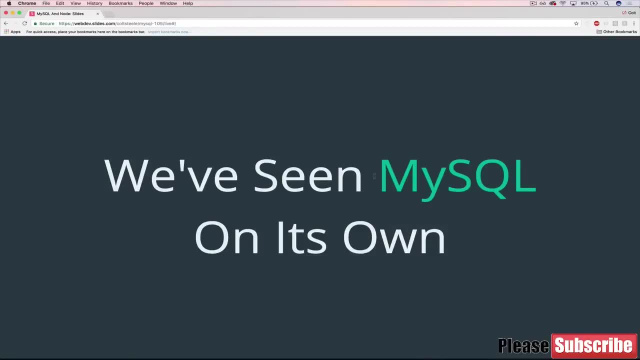 what we're doing and then, in the next section, we'll build a web app to connect to our database. all right, we're almost there, all righty. so, as I mentioned in the previous video, this section is a big turning point and hopefully you're excited about it. I'm excited to teach it. we're going to go from what we've been doing for the last 12, 13. 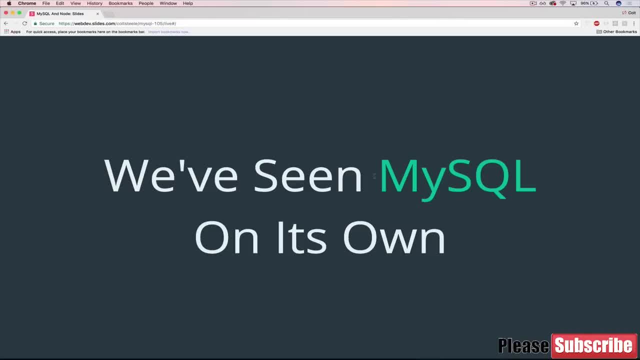 ish hours of content, basically working with MySQL on its own, querying a database and getting a result printed back to us immediately, which is great, but we're gonna go from that to creating applications with MySQL. we're not gonna, you know, learn how to create complex video games. 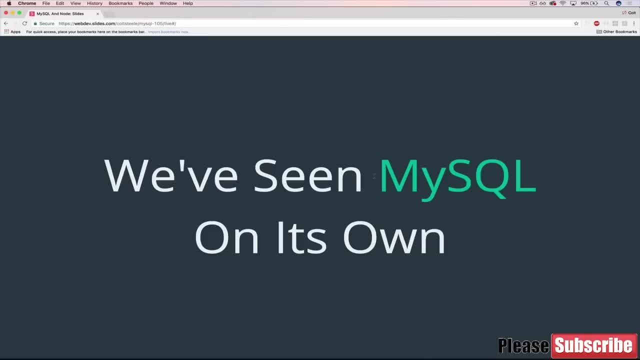 or or crazy iOS apps. we're focusing mainly on web applications, but the ideas are the same. I'm going to show you how you get an external language like JavaScript or PHP or Ruby to talk to MySQL, and we'll build a couple things with that. now let's quickly review what we've done- not the entire. 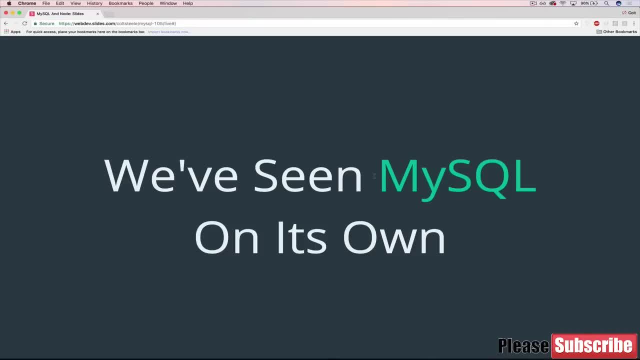 course, but the way we've been working and talked about the merits of that. so we've been working with the CLI mainly, you know, having a database of users or books or whatever it is, and asking, selecting sales data or orders data or customers, and trying to figure things out like you know how. 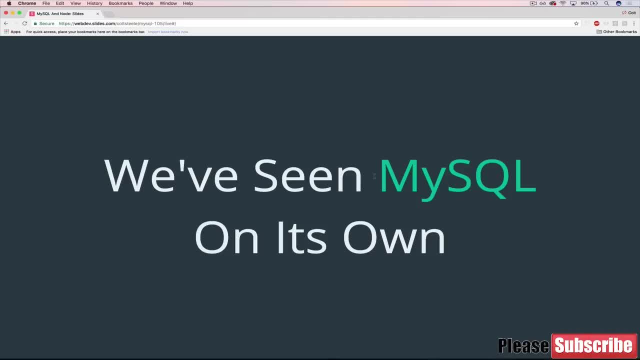 much did we sell last week? or what day of the week was our best-selling day across the last two years? those are really important and valid and just common uses of my SQL. so there is this whole subset of creating applications that we're diving into now, but there are tons and tons of jobs- lots. 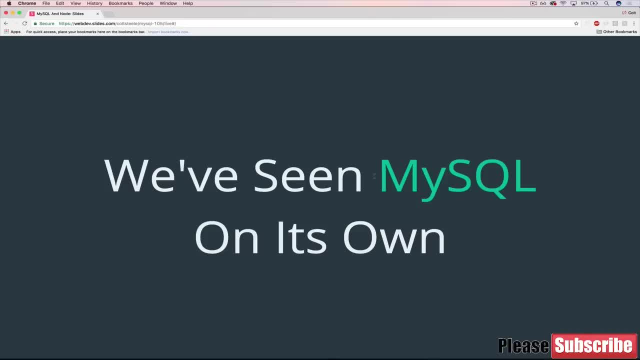 of people who, when they work with MySQL, all that, they do not to diminish it in any way, because they complex queries, but they're working with only MySQL and they're opening up the CLI or they're writing SQL files, like we've seen, and they're just saving and running those files. So they want. 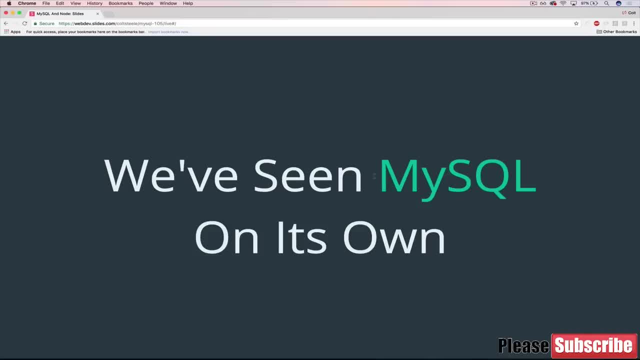 to see. okay, what was my commission that I made in the last year? Calculating tax, whatever information, summing a bunch of information in these tables or doing a complex join to figure out which promotion worked the best. Those are really important and common uses that people do. 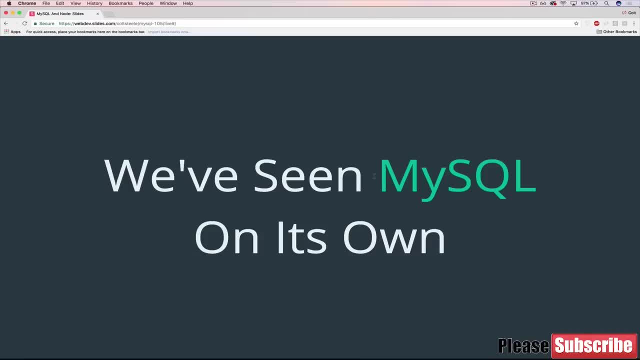 all the time. So it's not just about building applications, but we've seen that first part. We've seen how to do that. We've worked with tables. We've been writing lots of selects, inserts, updates, deletes, all of that. Now we're going to see how we work with other languages. 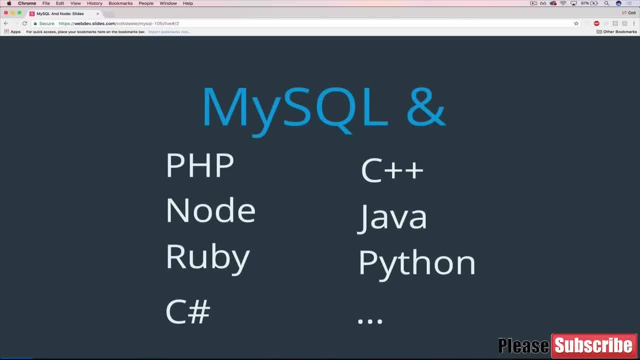 So now it's time for MySQL plus. any of these, pick one, And the reason I'm even showing you this page is not to intimidate you, not to make you think you need to know all of these. You only need one. So, depending on what you're doing, there are strengths and 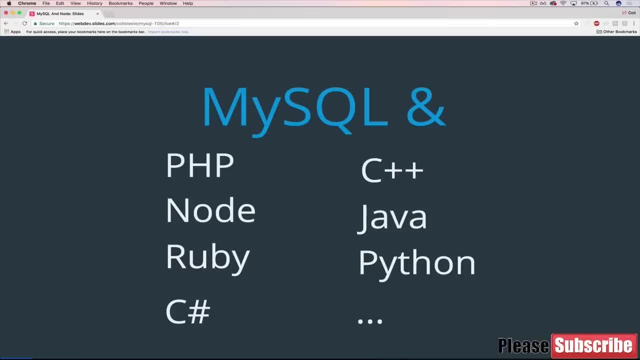 and uh, disadvantages to certain languages, Um, but really all of these will work. They all have ways of communicating with MySQL. So if you're someone who is comfortable with a language, like if you grew up working with Java or you took a Python class in college or whatever it is, 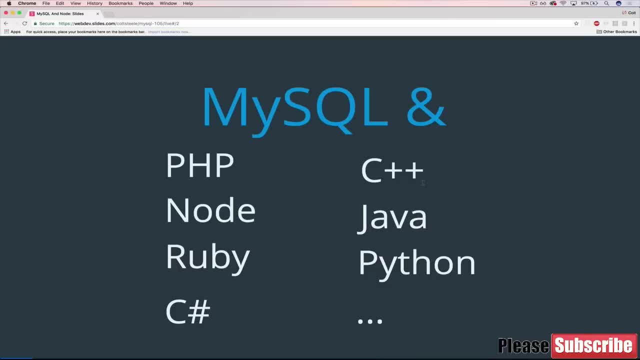 you can find ways, I'll. I'll talk about what they are- of connecting MySQL and whatever language you're comfortable with. The one we're going to work with is called node node JS. It's, uh, getting very, very popular. It's been pretty popular. It's been very popular for a long time. 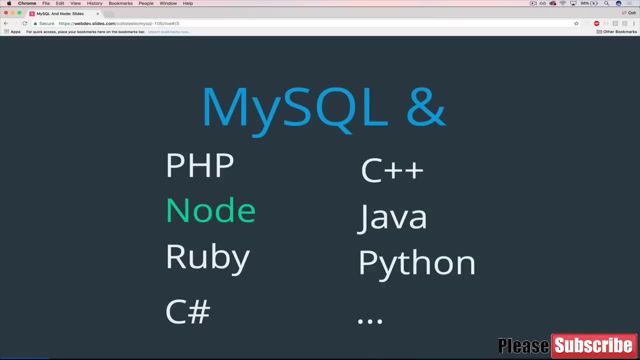 Very versatile language. lots and lots of users- uh, great documentation out there. Now we could have also gone with PHP. Some of you may be wondering about that. PHP and MySQL historically have been a bit of a an item. a couple, uh, that are: 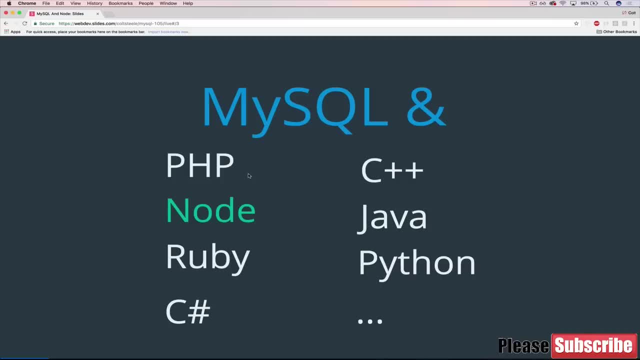 uh were spotted together all the time. In the next video I will talk a bit about PHP. It's totally optional, but I didn't want to bog you down in this video with it. but, uh, there are a lot of opinions out there. I'll give you a 10 second preview. 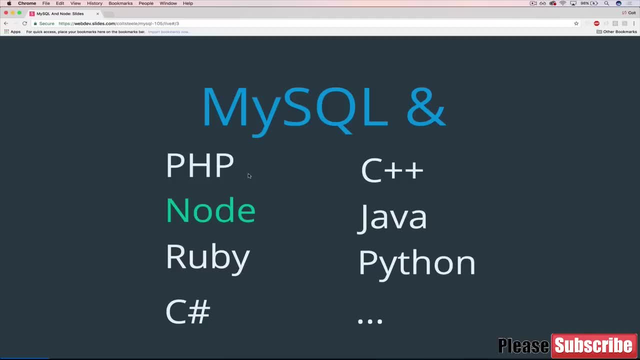 A lot of people think PHP is dying. It's certainly in decline compared to where it used to be. It used to be the king of programming languages on the web. Now there are lots of competitors and people are leaving PHP. It doesn't mean that it's a bad. 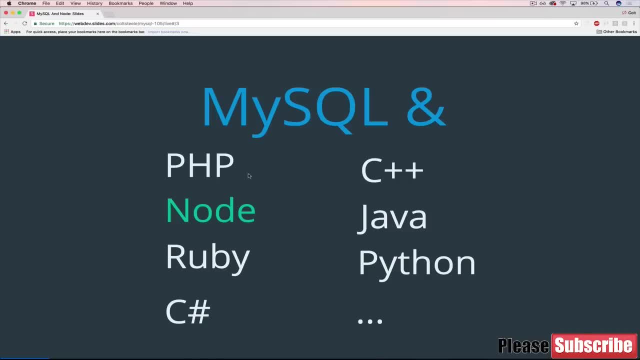 language. There are problems with it. This is my opinion as well. There are problems um that other languages have been able to solve better. However, there's a big user base out there. Yes, it's not growing as fast every year, but there are still. 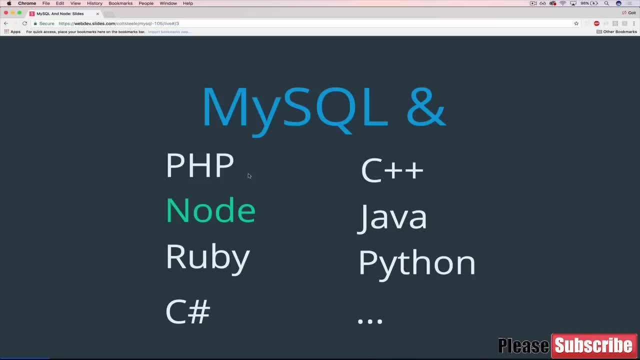 million to people using it. So do not shy away from PHP If you're comfortable with it, if you want to use it. there's lots of examples out there, But I didn't want to make this course just another PHP and MySQL course. There are dozens. They're getting dated, but there are dozens of them even on Udemy. Lots of MySQL and 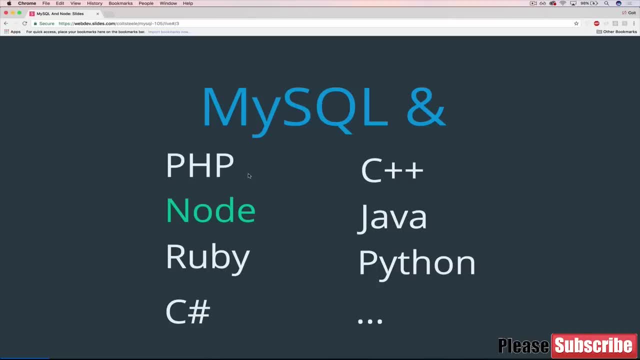 PHP. So I chose Node and I'll talk more about why in this optional video coming up. Basically, JavaScript is the most popular programming language for the web right now and Node uses JavaScript syntax And just generally. Node is a great choice And I 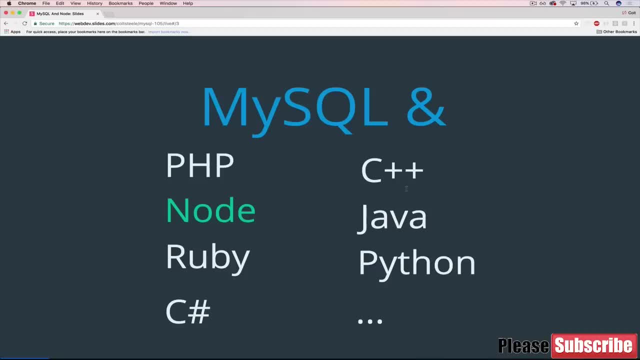 could have gone with any of these, although I probably wouldn't have done any of the C languages, But Ruby or Python would have been equally good choices. However, I went with Node because, honestly, that's what people want to learn right now And it's what a lot of the jobs out there are for. 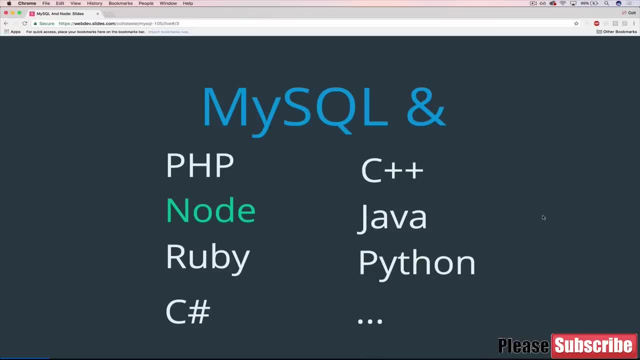 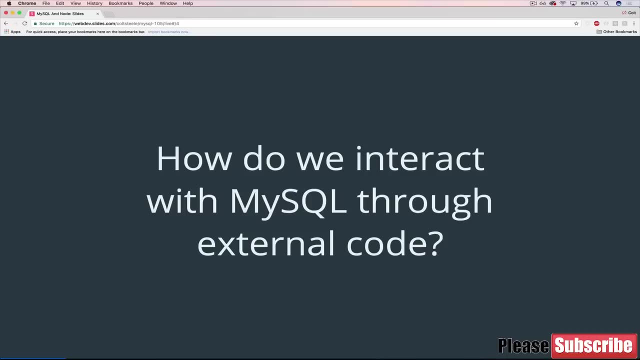 Okay, so that's all I'll say about that. for now, Like I said, any of these will work. The next thing I want to talk about is: how do they work? What do they do? So we pick a language, we're working with Node, But then what? What's the point of, you know, using a program? 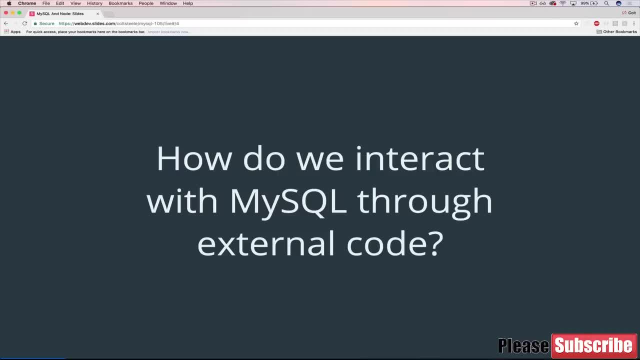 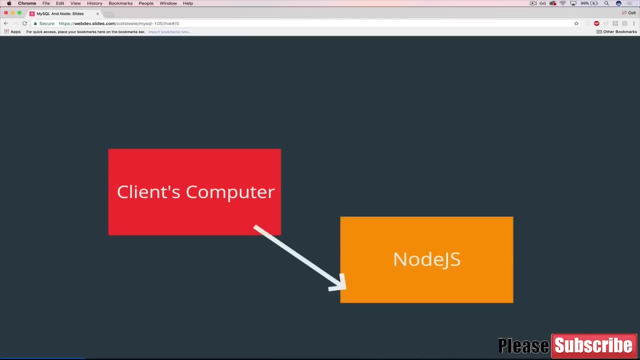 programming language. how does it talk to mysql through external code and what kinds of things would you do? so here's a little diagram. imagine that there's a web application. my computer when i go to this is hypothetical amazoncom. i hit enter, a request is made and i label this as node. 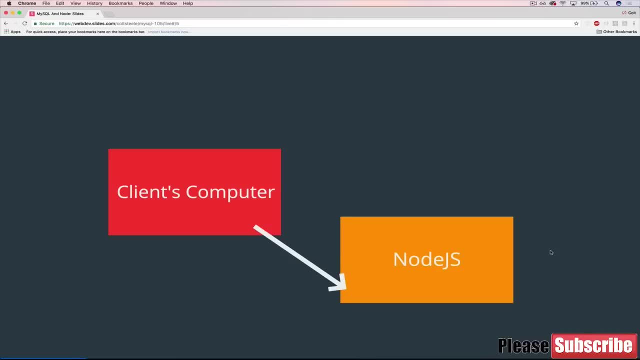 js. amazon does have some node in their stack, but this could be any language, so that doesn't matter. but i send a request. hey, amazon, can you give me your home page, or can you give me, uh, my personal profile page? i want to update my email address, how about that? and then the code: whatever it's. 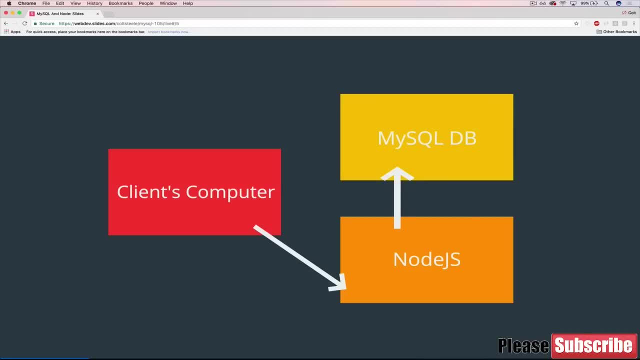 written in is going to talk to mysql. it's going to say: hey, mysql. uh, this user with the you know user with the email of colts at gmailcom is trying to get his profile page. i want to select all information related to you, or you know. select everything. 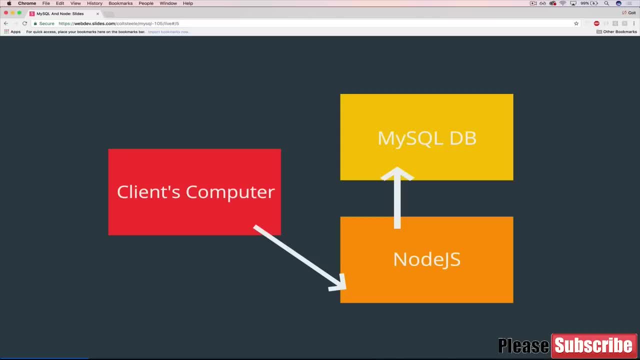 from users. where email is called to gmailcom, that query is run. so from node or whatever this is here to mysql and a result comes back. and it could be. i'm sorry there's no users table. i don't know what the heck you're talking about, node or it could be okay. here's the five items in that row. 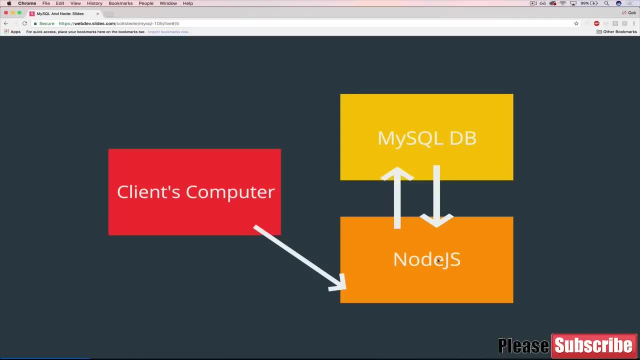 about colt, and then that comes back. so that's kind of this two-way street, and then whatever the programming language is here is then going to compile whatever sent to me, so the amazon home page. so it's going to take all those results and it's going. 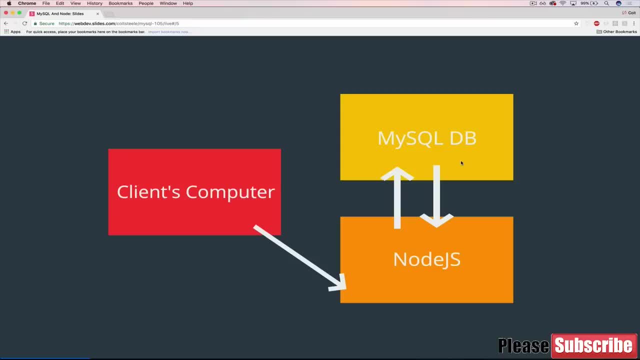 to build a web page for me and send it back. now. this is not a course on web development. i have another video where we talk about what this course is and isn't and how i'm going to go about covering things like html and css. i'm going to cover them, but not in a ton of detail because that would could. 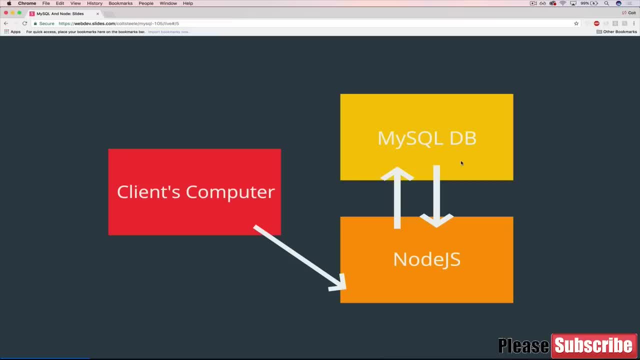 take hours. i have a 45 hour course on that content, so this is really more focused on the mysql part. makes sense. it's a mysql course, okay, so with that said, oh, i missed the last arrow. uh, something is sent back to a computer. so it's a cycle where there's kind of three entities, there's a device, 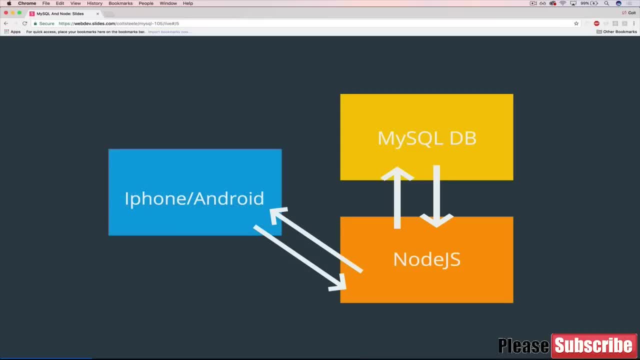 over here my computer. um, it could be an iphone or android phone, could be- uh, i don't know. it could be a smoke detector. it could be a nest camera. if you have ever seen nest cameras or any like web-based security camera, they don't. i'm not saying they work with node and mysql, but there's. 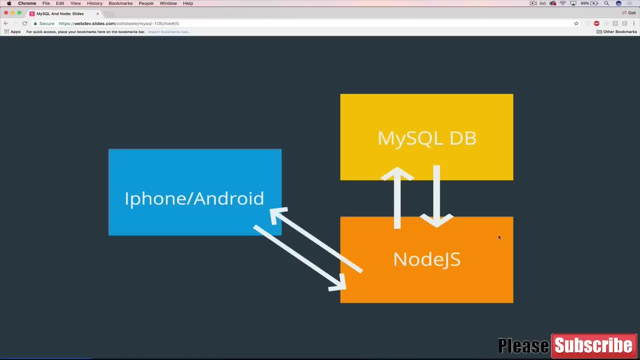 somewhere storing information and there's some app somewhere running that is listening, that's getting video sent back or updates from a smoke alarm, um, or it could be a virtual reality headset. it could be anything, really any sort of device, uh, another computer, a phone, something else, and then 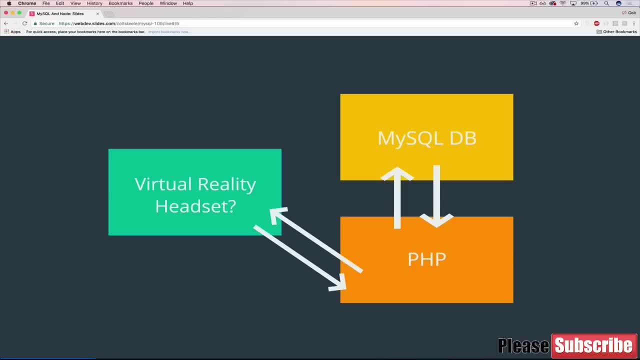 this here, like i said, doesn't have to be node. that's what we're working with. but you could easily replace that with another language, php, or ruby, um, and then, yes, you could have a different database, but that's not what this course is about. but you could, you know, have a virtual reality headset. that's working with ruby, although that's. 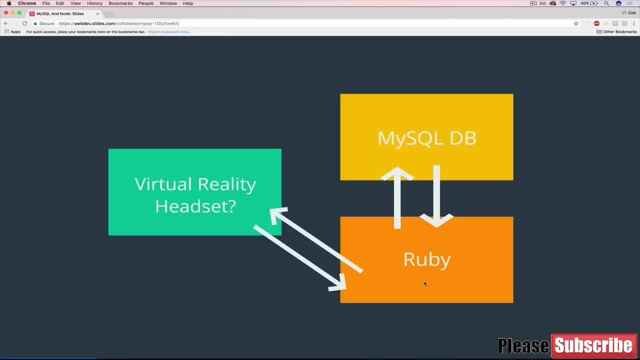 not a great game development environment. maybe you're working with unity and you're writing java or something, but then you're working with another database. it could be anything mongodb, postgres or mysql. the core idea is the same. okay, so that was a lot of talking. like i said, there's an optional video coming up about php versus node and other languages. 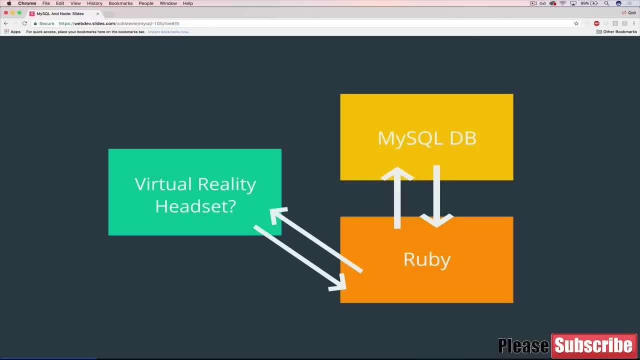 it's mainly my opinions, but there is some interesting data to tell you about. so if you're interested in looking at this and if you're interested in learning about the php version, then you're probably going to want to take a look at. if you're curious about, you know how i came to. 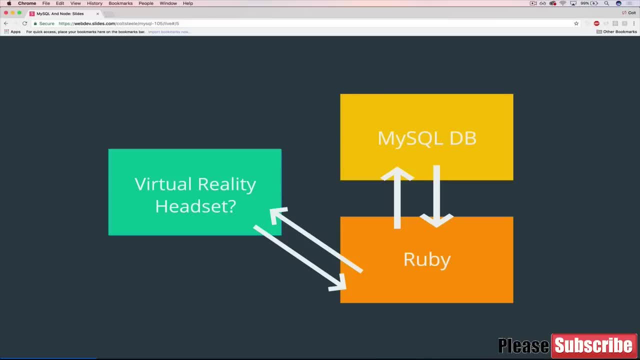 the conclusion i came to. i spent a lot of time thinking about how to teach this, and what i'd like to do is add kind of alternate versions of what we're going to build here, and build a ruby version so you can see it, and then build a php version and build a java version so you can compare. 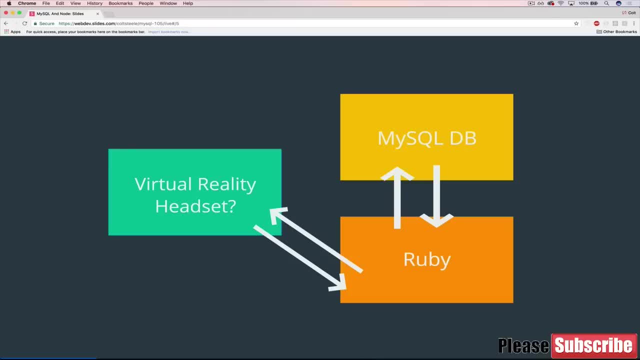 it, but that will come later. this is, you know, i made a decision and it's an informed decision and i'll explain why, if you're curious, in the next video and then after that, or you can skip the right to the next video, which is going to be introducing the project we're going to build. 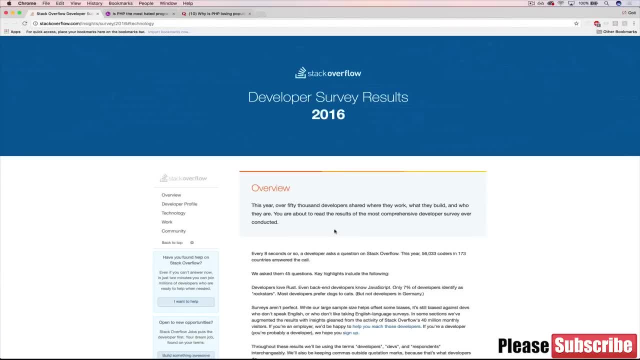 all right, so i'll start this video off with a quick anecdote, stupid story. i have a course online right now. it's done relatively well, a lot of students and it focuses on a bunch of technologies, including html, css, javascript. we talk about nodejs as well. talk about mongodb. 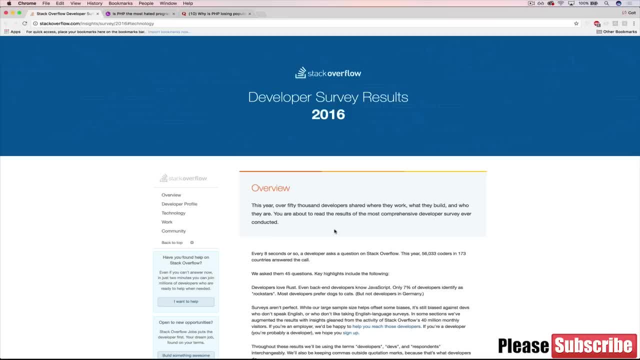 and a bunch of other tools that go along with them. and at least a couple times a day, you know, i get comments or questions or people demanding that you know it should cover php, or should cover ruby, or why doesn't it cover c or java? and those are valid questions, right people? 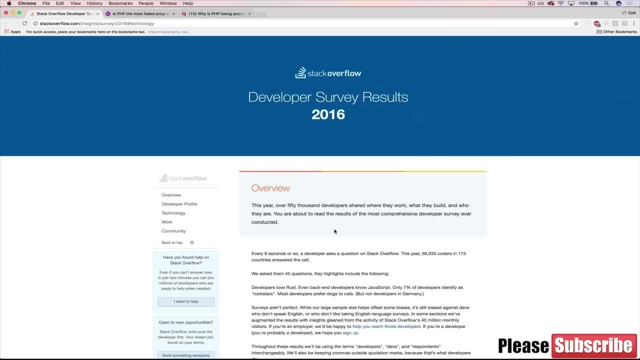 have reasons for wanting to learn different things. so i'm not trying to diminish their concerns or you know not. i'm not trying to say they shouldn't want to learn those, but there's no way that any course can teach all of those and there's no reason that it should because, like i, 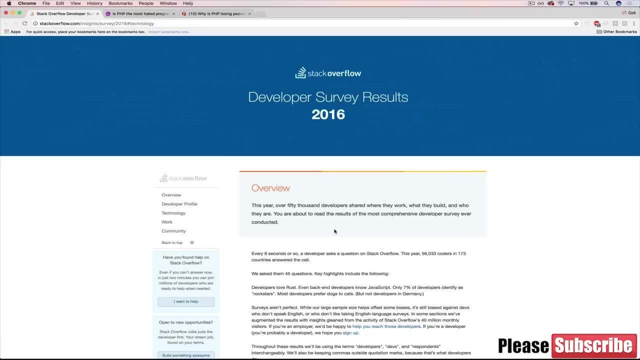 said you only need one, maybe two. so the reason i bring that up is that it's kind of a contentious thing. people, especially students, when people are learning to program, it's overwhelming. everyone tells you to learn something else. it's very confusing, you know, do you learn something? 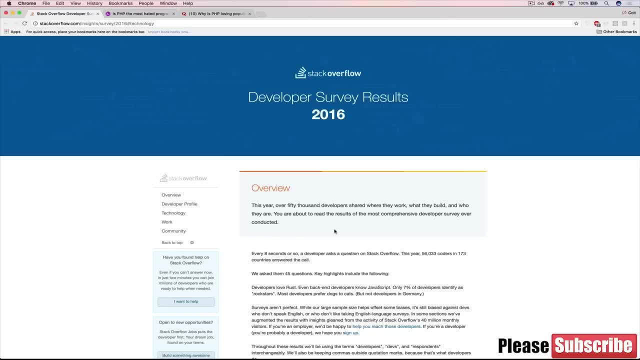 that's easy to learn because it's easy to learn, or is it better to learn something that's popular and more people are using, even if it means that it's tougher? you know what's the best route, and i think the answer is: there's a different way for everyone. it's kind of a lame cop-out answer. 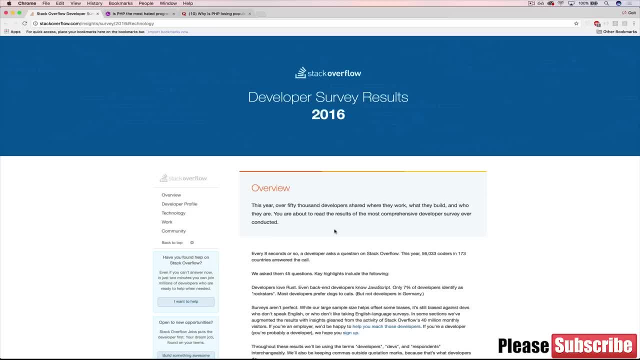 so when you're making an online course, you have to decide, and what i decided for this course is we're focusing primarily on node, and the typical kind of conventional choice would be php. so i want to talk about why i made that decision, and the first reason is that i personally am not crazy. 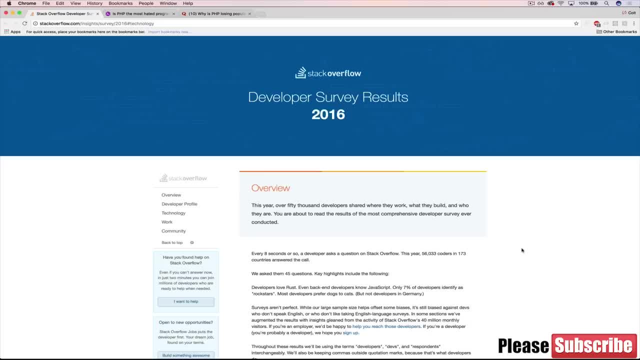 about php, yeah, i've done some work with it, some work with wordpress. it, like i said, used to be very popular. there's still a lot of people using it, but it is no longer the reigning champion of programming languages on the web, but more people are using it, and i mean as a professional. I like to say that php is a 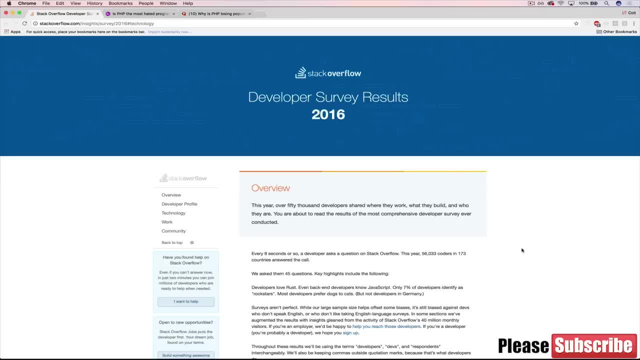 really good tool for me and it's one of the reasons I built it. like 7 years ago it was, that was the language that you use if you wanted to make a web app. but nowadays there's so much more competition. people are writing things in node or they're writing them in ruby and tons of other languages. 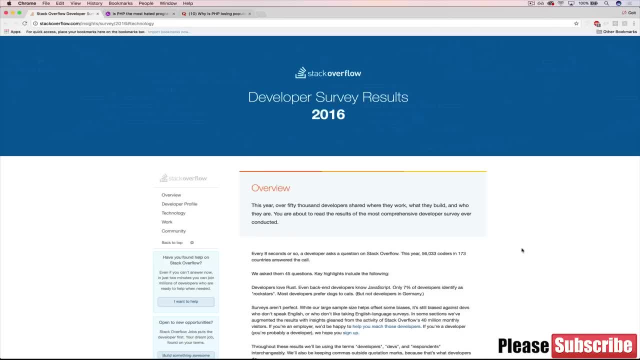 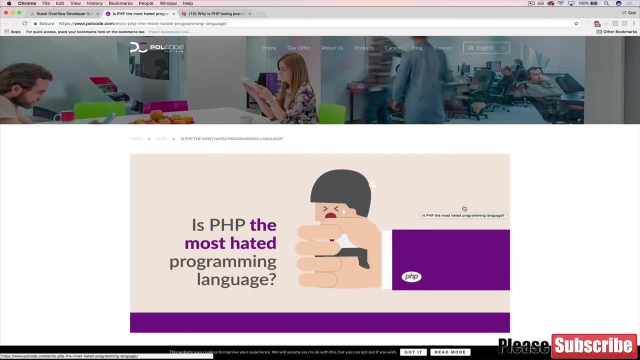 scala closure. all these different languages that you could use and they all have benefits, right, they all have kind of. they came later they were able to see what worked, what didn't work. where I won't go into a lot of the technical details, There's an interesting article online. Is PHP the? 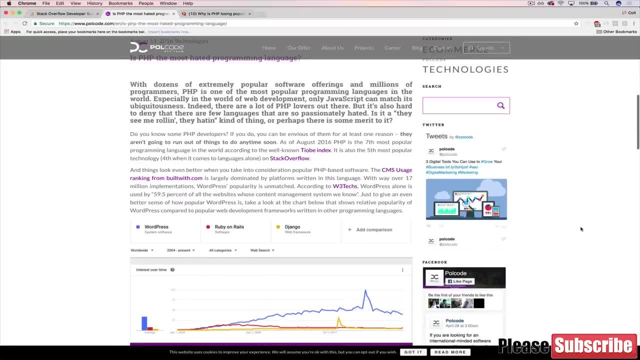 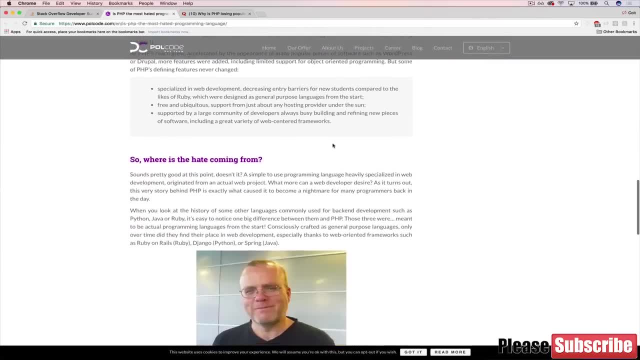 most hated programming language. Not that that is an excuse to not use it, but it's interesting. I'll link to it if you want to read about it. It basically talks about how PHP got so popular. back in 1995 is when it started. And then where does the hate towards it come from? 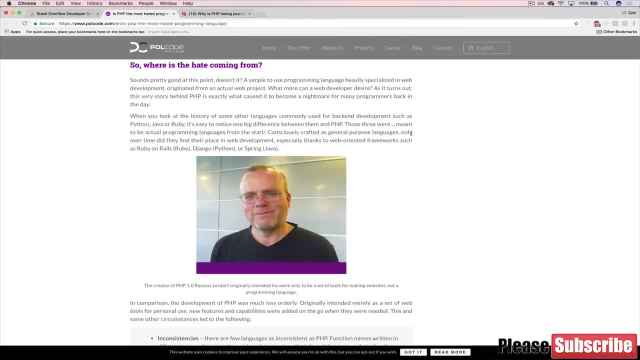 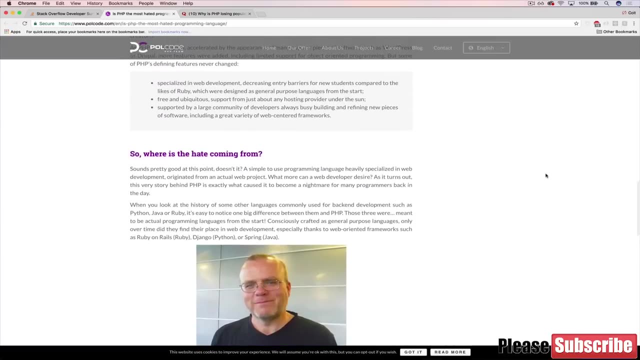 And largely the consensus at least, is that PHP was kind of cobbled together. It wasn't a consciously crafted- as this says here- programming language. Things were added over the years And there's inconsistencies, There's some security issues, But you could actually say the same thing. 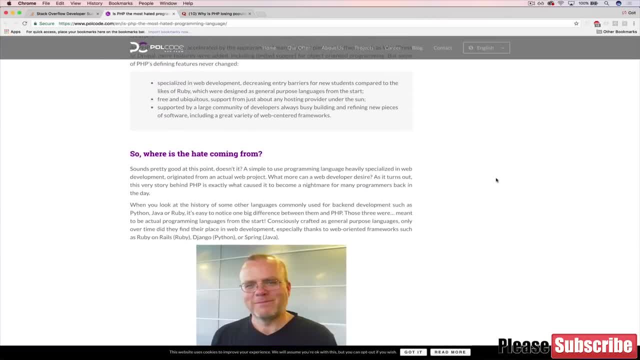 about JavaScript, which is a valid criticism, that it was created in I think it's nine or 10 days, kind of as an experiment. It wasn't some crazy planned out. language and things have been added And it's not a valid criticism. It's not a valid criticism. It's not a valid criticism. 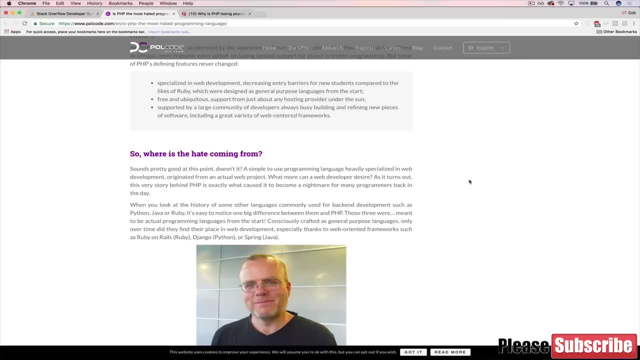 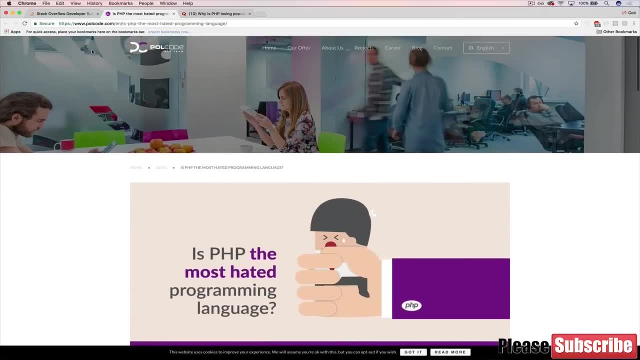 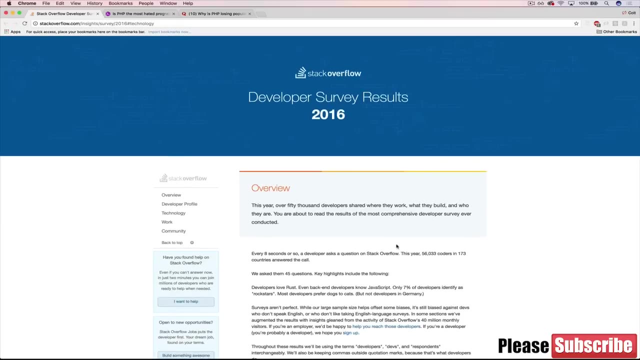 And they're constantly kind of updating the specification for JavaScript, So that's not necessarily why I chose to not teach PHP and choose Node and JavaScript instead. It's really more about the data that's on this page. This is from 2016.. It's a Stack Overflow survey, they do. 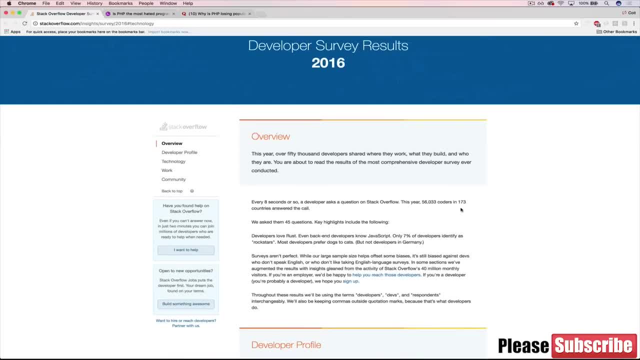 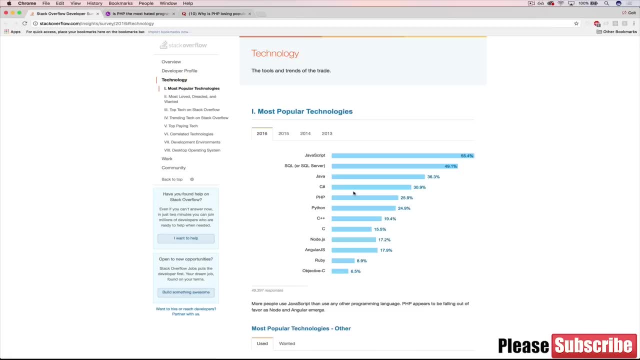 with how many- 56,000 coders who answered the survey, And there was 45 questions. So if we scroll down- I'm going to click on technology and go look at the technologies tabs- We can quickly see, first of all, SQL- very popular Good news, And you can see here we have PHP which is in. 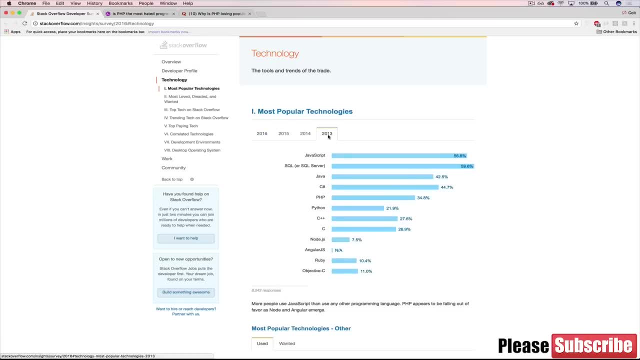 2016,. around 25%. If we go back to 2013,. notice that it started at 35%, then went down to 28%, then up a little to 29% and then down to 25%, so the lowest it's been. So you can see. 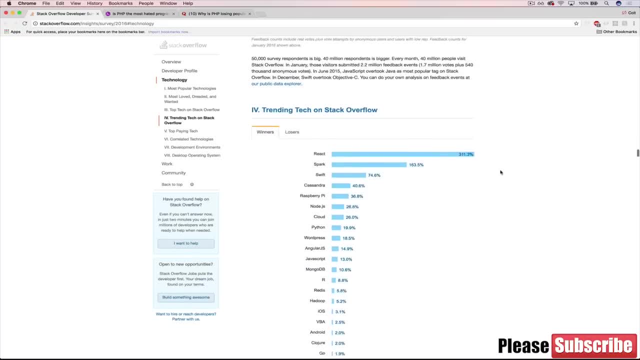 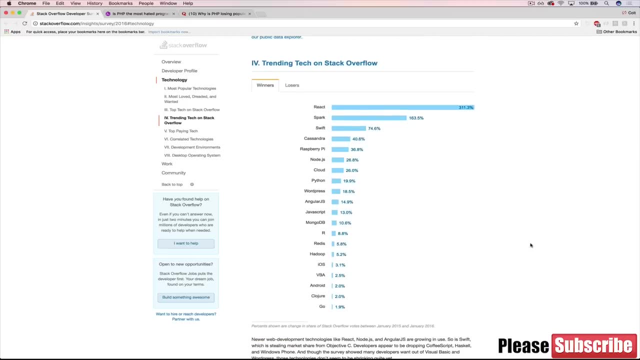 there are charts online that I couldn't find any that were copyright-free, essentially that had a license that I would be able to show you the image. But there are charts online. You can see the decline. It's not a very steep decline, but there is a decline. And at the same time, if we look at 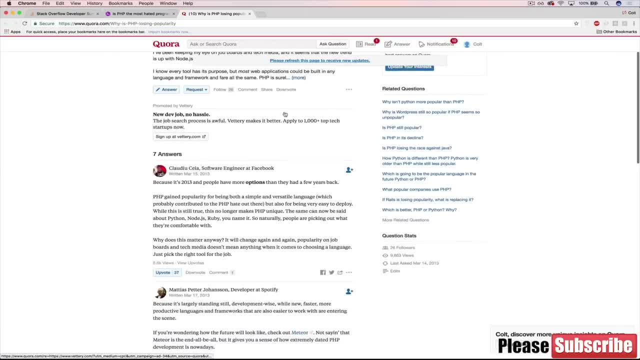 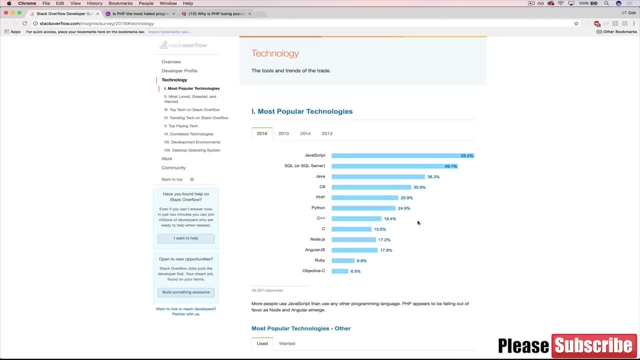 Nodejs here, which was at 7.5%, now it's going up to 9.9%, 13%, 17%. It's growing very quickly in comparison to other technologies. So it's growing very quickly in comparison to other technologies. 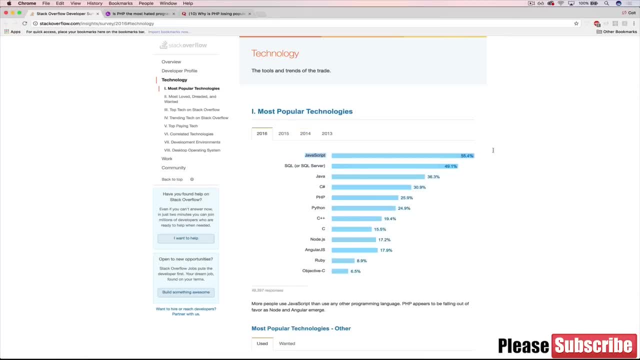 So it's growing very quickly in comparison to other technologies. So it's growing very quickly in comparison to other things around it. And then also, if you take a look, JavaScript is up here as number one, which is great because Nodejs uses JavaScript syntax. It is JavaScript. We'll talk. 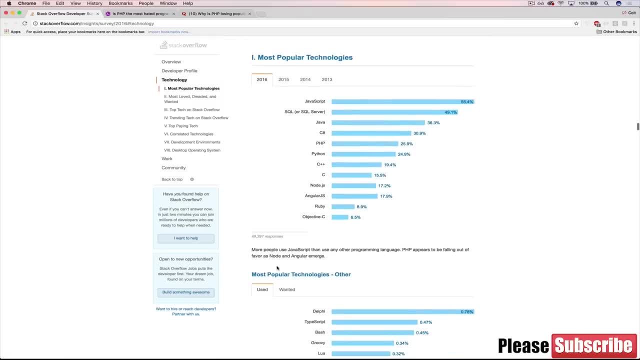 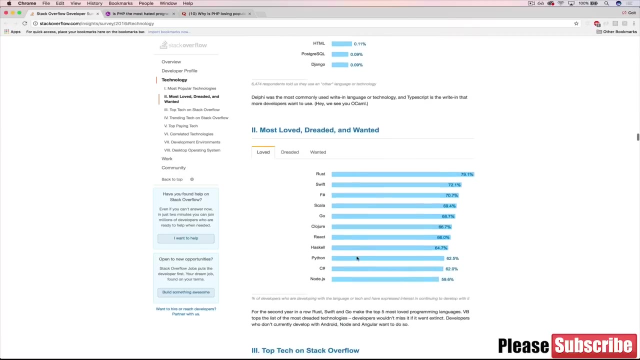 about that if you're not familiar with it. So if you notice the trends down here, more people use JavaScript than any other programming language. PHP appears to be falling out of favor as Node and Angular emerge. That's kind of the main takeaway trend And if we scroll down a bit more, we can. 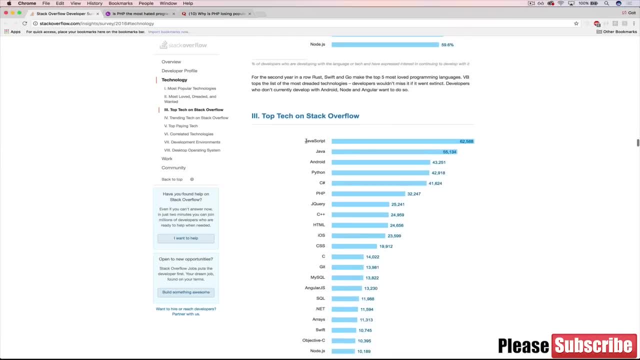 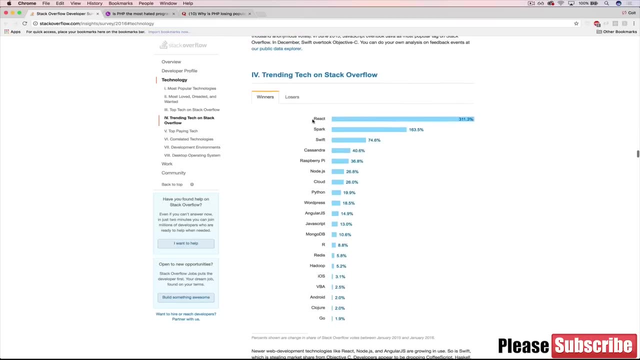 take a look at Nodejs. The top tech on Stack Overflow can see JavaScript up nice and high still. If we look at trending stuff, you'll basically see that it's all JavaScript. well, almost all JavaScript related React is JavaScript. We've got Node. Nowhere on here is PHP. Now I don't want to say that you. 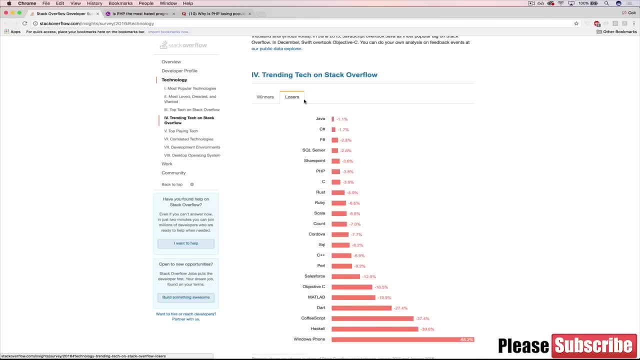 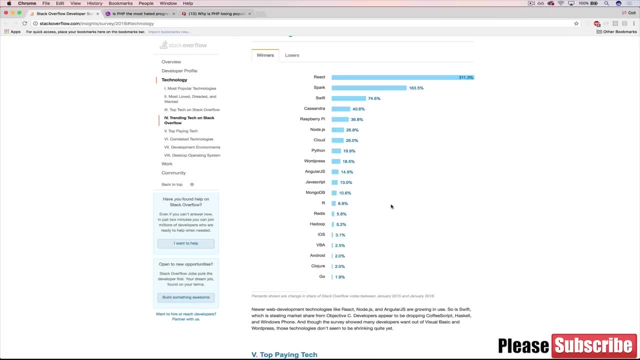 only pick something based off of if it's trendy or not. That's not the point here. The point is that I picked Node because it is something that will prepare you for the future, And if you want to learn PHP, there are so many options out there. 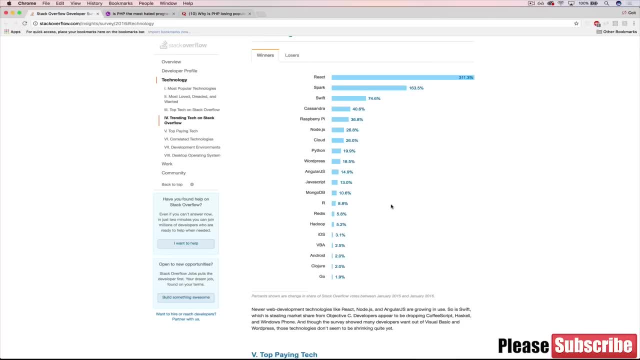 And I didn't want to just make another version of a course that could have been made a couple years ago. I wanted to make the most up-to-date current course. So basically, it's a decision that I made. There is not one answer. 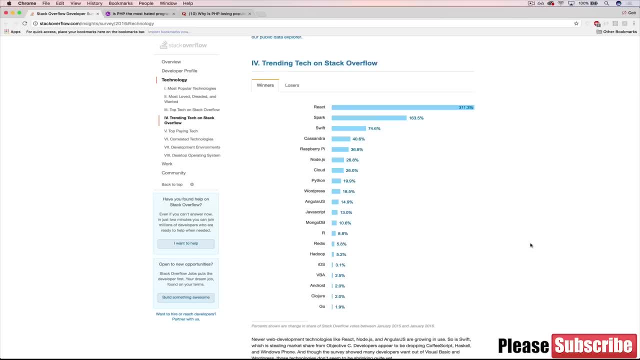 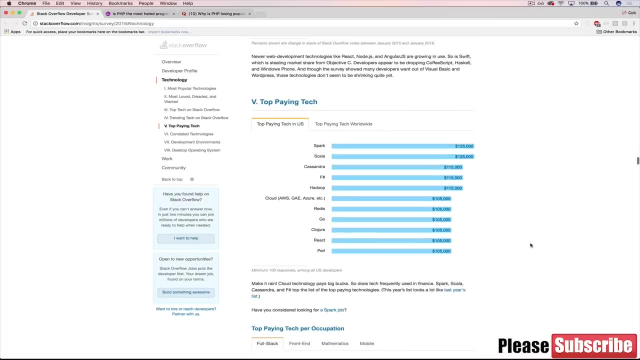 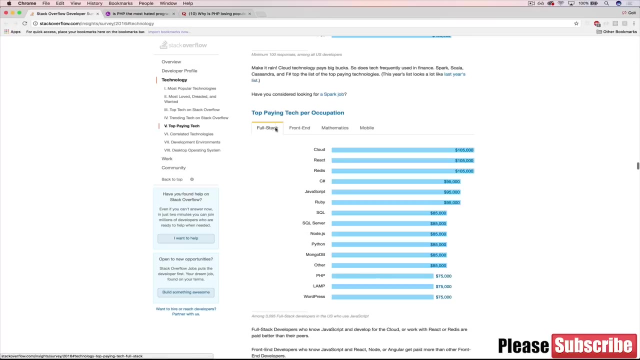 You could still make a great PHP and MySQL course today. I'll probably end up adding a little PHP section, but it's not going to be the focus of the course. And minor, minor thing, but it is interesting if you look at your top-paying jobs or if you scroll down and look at what a node developer on average is- around $85,000. 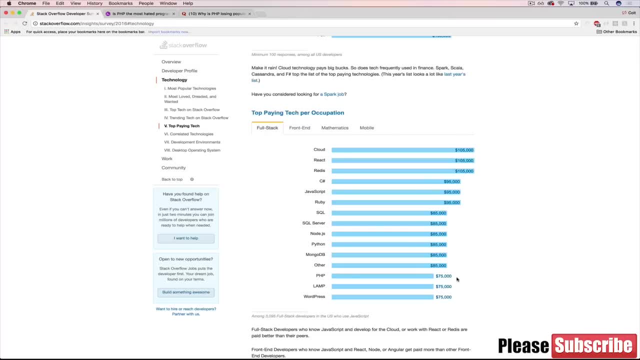 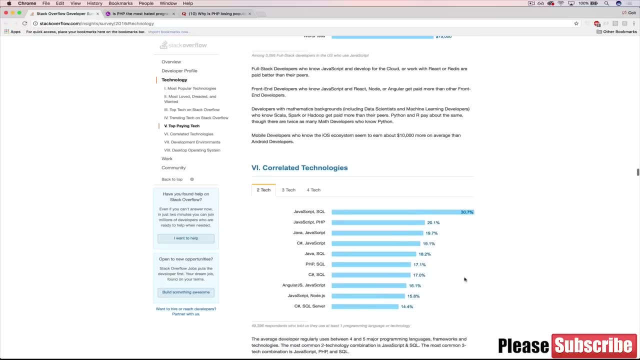 You look at PHP, minor- well, $10,000 difference. So not that that's why I chose to do that, but it is interesting to see. And then, finally, if we look at the correlated technologies, you can see PHP and SQL. 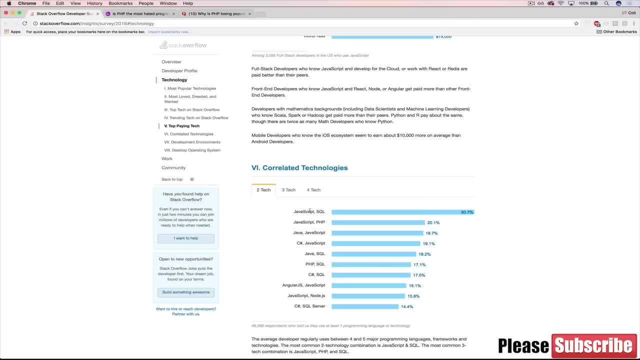 There's a tight correlation there, But there's also JavaScript and SQL, which is what we're going to be focusing on, And that's becoming very, very popular. a great combination. So that's sort of some of the data behind why I picked that, why I came to this decision, if you're curious about it. 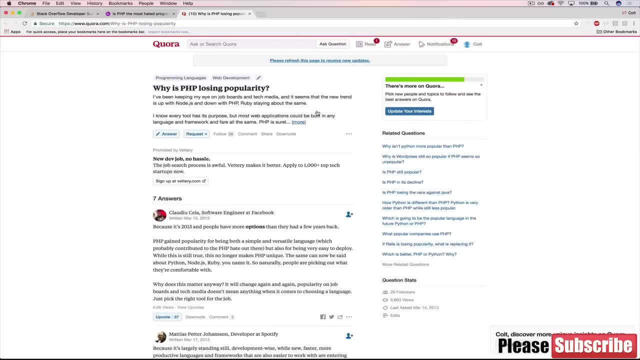 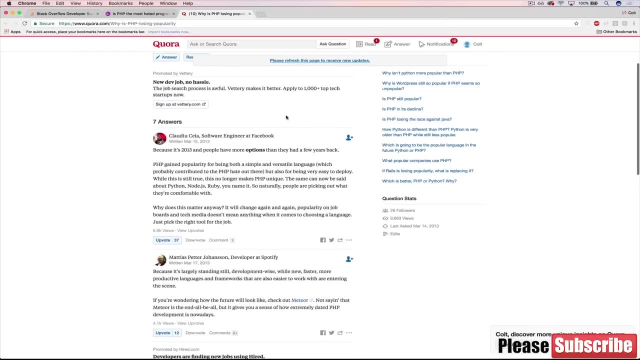 One other thing: there's a good Quora post about why PHP is losing popularity, why people are trying to do Node and stuff and Ruby and why people are down on PHP, which hopefully the takeaway Is that that's not my intention, is that I'm not trying to make PHP seem bad. 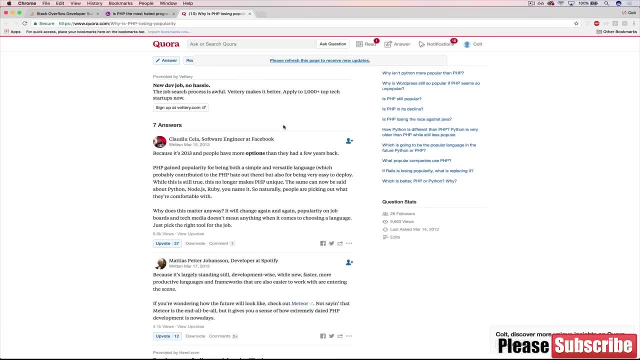 I am just trying to show you another option. All right, So thankfully this was an optional video. You didn't have to sit through this- and not that you have to sit through any video- but well, we're done with it now. 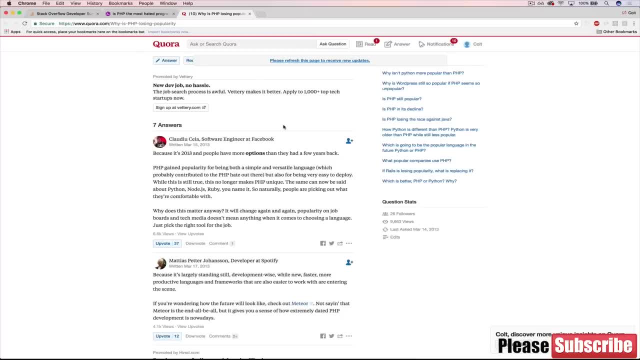 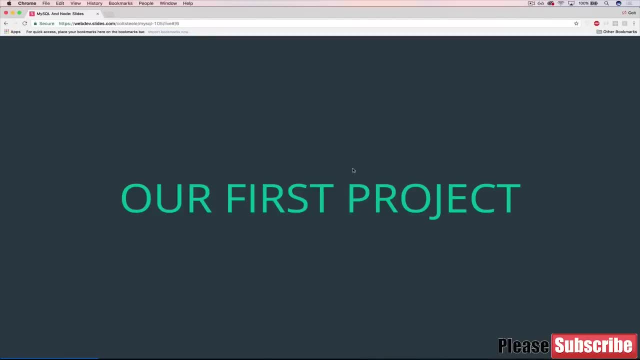 Thanks for sitting through that. if you chose to Next up, we're going to introduce our very exciting fun project. All right, So we're back. If you watch that optional kind of boring video, we're now moving on to an exciting and non-optional video which is all about the. 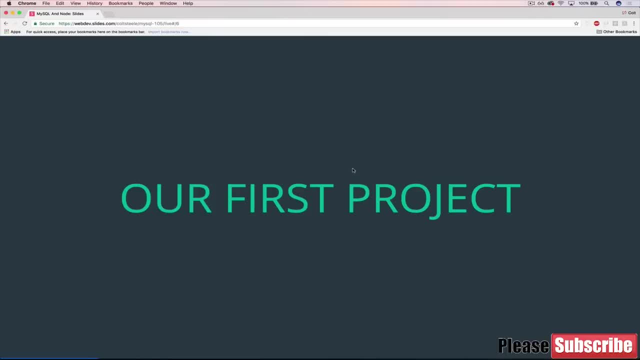 project we're going to make. So we're going to build a simple web app to start using Node and MySQL together. So what is this app? Well, it's called Join Us and it's a cult mailing or, excuse me, a startup mailing list application. 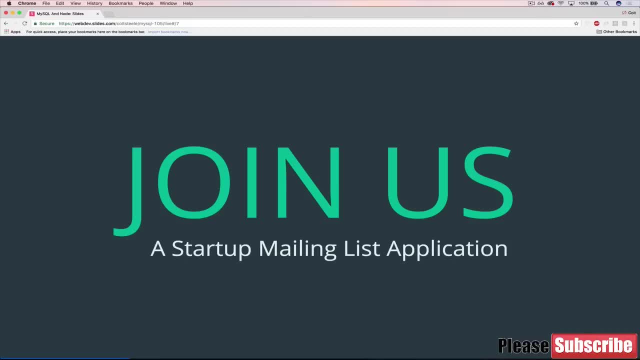 So it's. you've probably seen this before when there's a new company that's launched. Maybe you haven't, but if there's a new company that's launched, they're not quite ready yet, but they want to get their name out there. 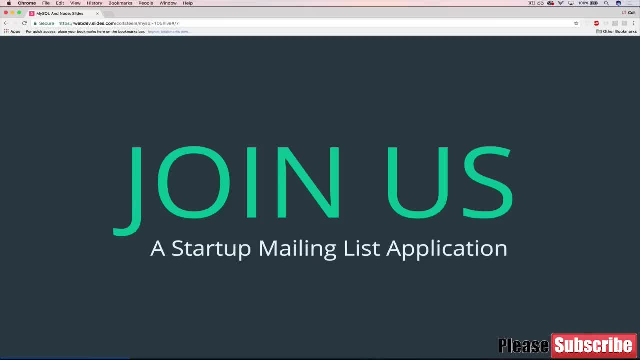 They want to start getting interested parties registered or collecting their information so that they can send updates or so they can invite them, you know, once the application is launched. So that's what we're going to build, Uh, basically a way of collecting people's emails, and it looks like this: 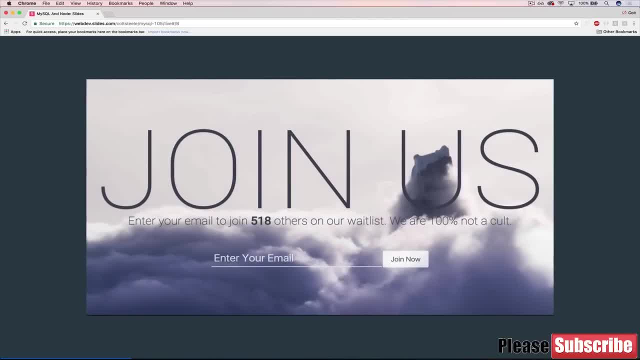 Now I'm not, you know, a great designer in any way. That's not the focus of this course. Hopefully you think it looks okay enough, but really, what I just want to go over are the different features. Now, it's not very feature rich. 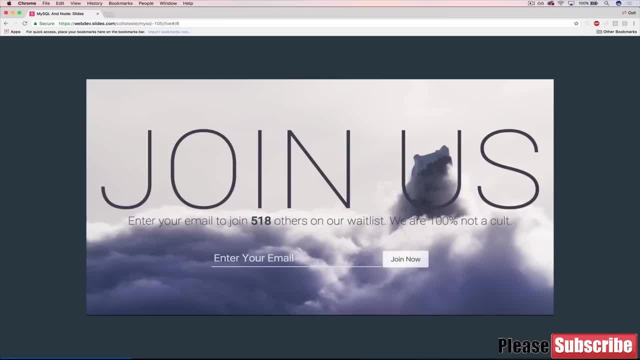 The point is to make something simple, but to show you how the we're connecting with MySQL- Yeah, Through Node- and how this application kind of showcases both selecting information and inserting information. So the first thing you'll see- there's a photo here and we don't have to worry about copyright or licensing issues. 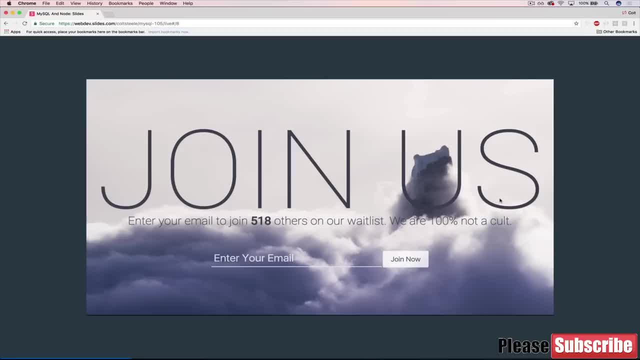 I actually took this photo. It's a bit of a brag, I guess. Sorry, Uh, but back to the content here. uh, we've got join us in big letters and then we've got enter your email to join And then a number here, and this number changes. 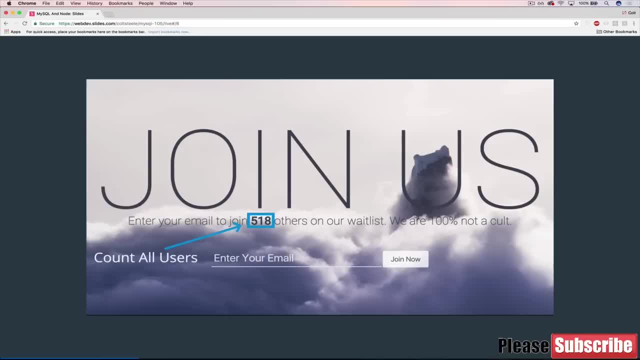 So 518 is basically the count Of all the users currently in our database. So when I made kind of this, uh, what will I call this? The alpha version that I made screenshots of that I'm I made before you know. I have to make the app before I teach it. 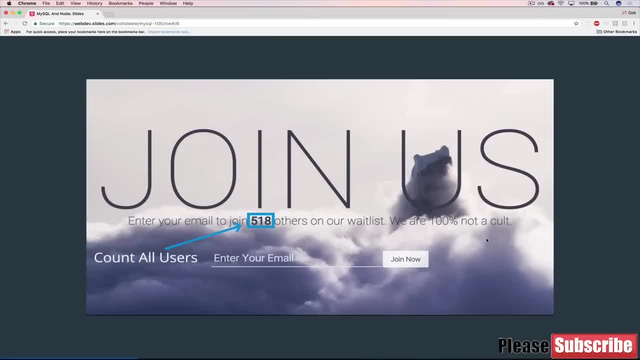 So when I made this version, I had 518 users in the in the wait list in the database. Um, we are 100% not a cold. Then the other thing is this: enter your email. join now button, which you enter an email. 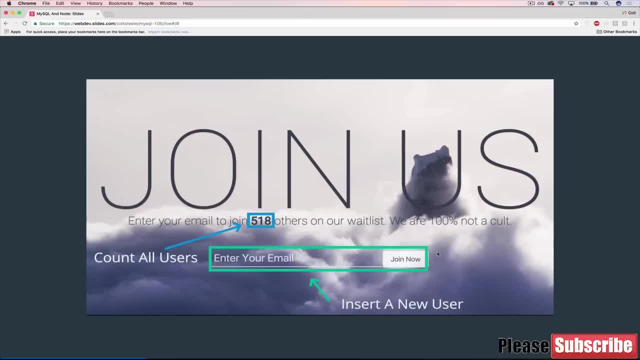 It's going to take that email address and insert, Insert it into our database. So there's kind of two things we're doing right: Selecting. we're going to count how many users are in the database. We don't need all the information. 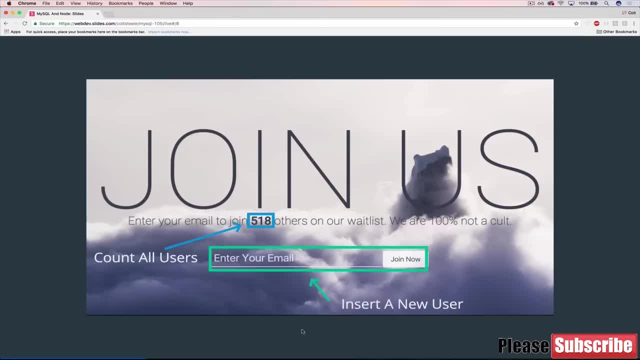 We don't need 518 email addresses, We just want to know how many. and then we want to be able to insert something from a form. When you click this button, it's going to go send the data to our node server. Then the node server is going to send it over to the MySQL database. wait to see if it worked or not. 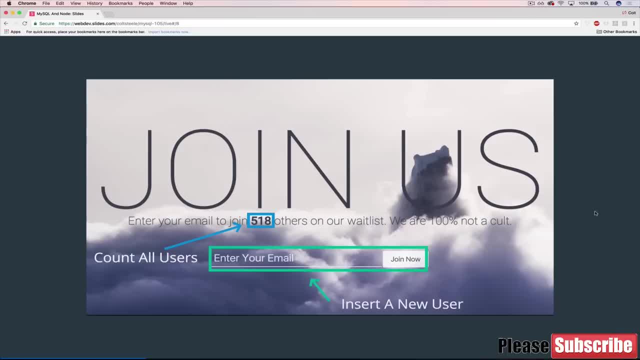 And then it will do something. you know we'll decide what it does. Does it take you to a new page? Does it just refresh the page? Does it show you a message that says you're signed up? whatever it does, Uh, but the key really is about adding information to our database and getting information out. 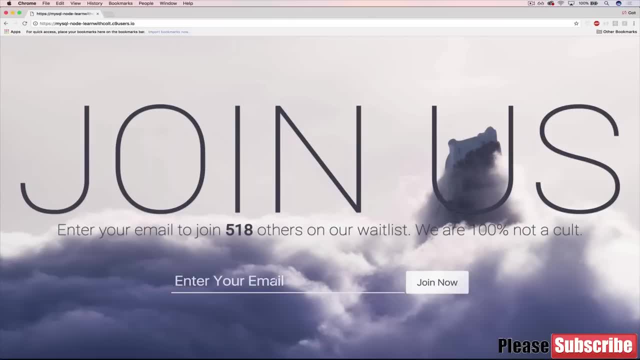 Okay, So that's how it basically works. Let me show it to you. Here I am. I've got join us. Let's create a new user here. Let's call it. uh, how about blue the cat at gmailcom? 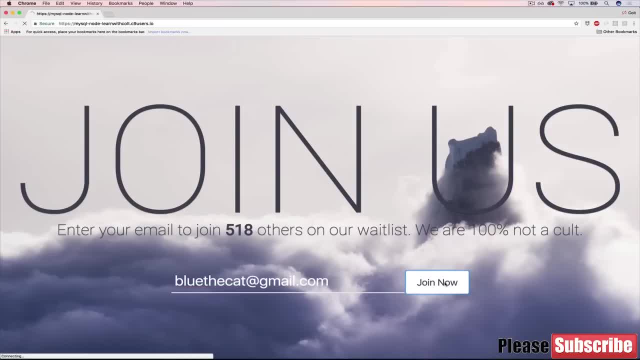 We click join now And you can see it takes us back, which we can decide what to do. uh, if we want to change that, I'll show you how. but now it says we've got 519 on our wait list and you know, I can refresh, I can stop the server, um, which we'll see how to do in a little bit. 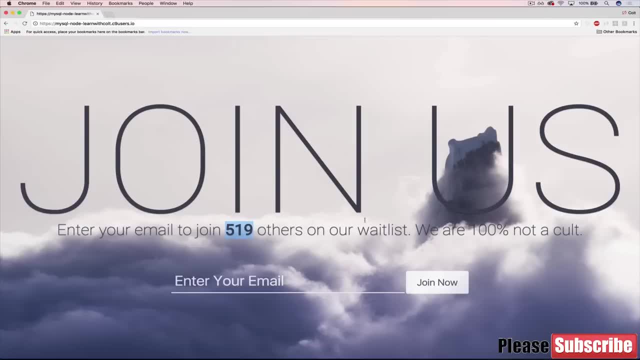 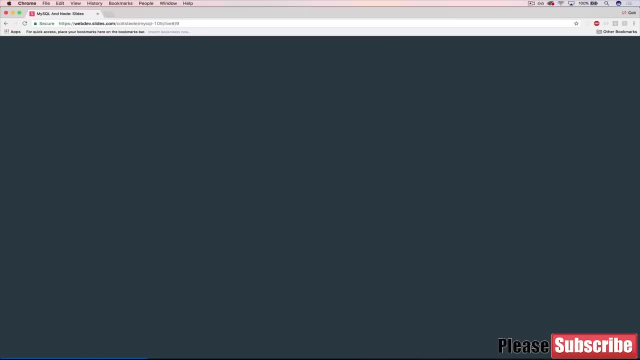 This will be 519.. This isn't hard coded in. This is coming straight from the database. Okay, So that's it. Now let's talk about how it works. What's the workflow like when I go on my computer like I just did? 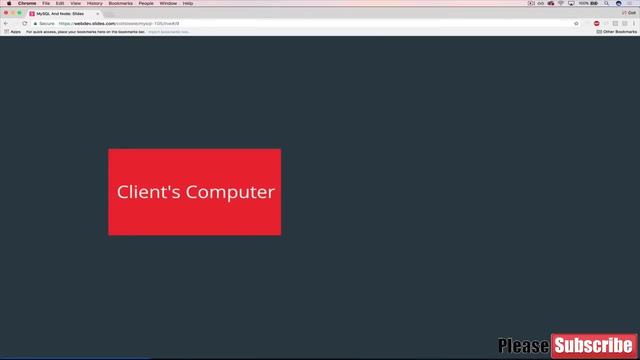 And I refresh the page, or I entered that address and I hit enter, a request is sent to our node JS server, which we'll see how to set up in a little bit, And the node JS server has code that says: oh okay. 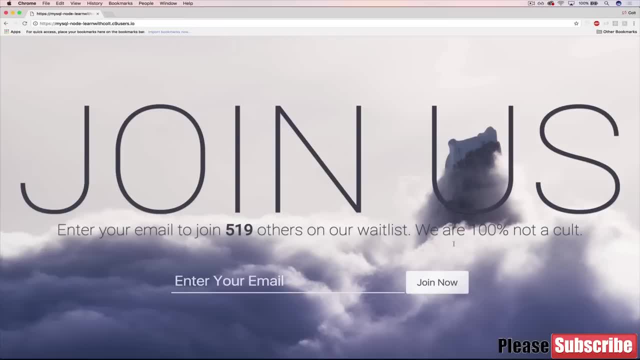 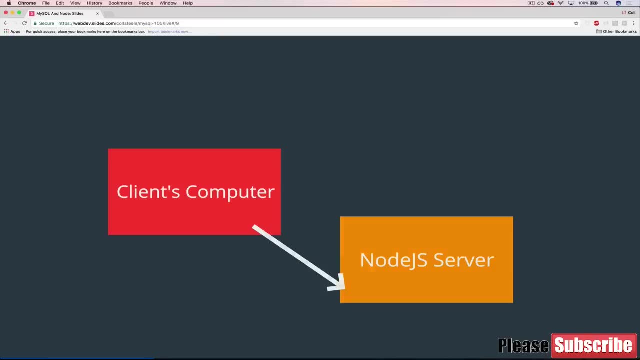 This client is asking for our homepage. Well, on the homepage we're supposed to have a number here of the total number of users in our database. So let's ask: Hello, my SQL database. Uh, can you tell me how many users are in the database? 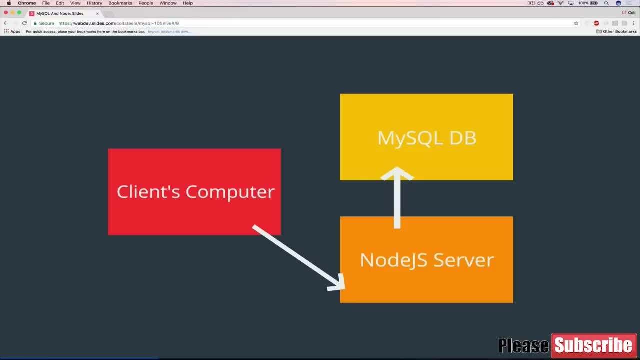 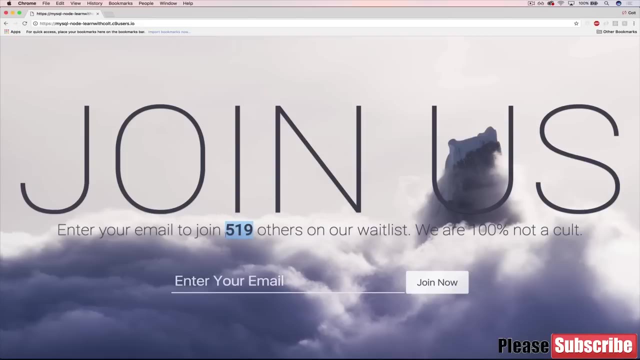 And hopefully You're aware that would be a count. So we do a select count star from users that will come back and we'll say ideally 518 or whatever it is, a thousand users. And then my server, the code there, takes that number and it plugs it in, puts it right here and it sends us. the page sends it back. 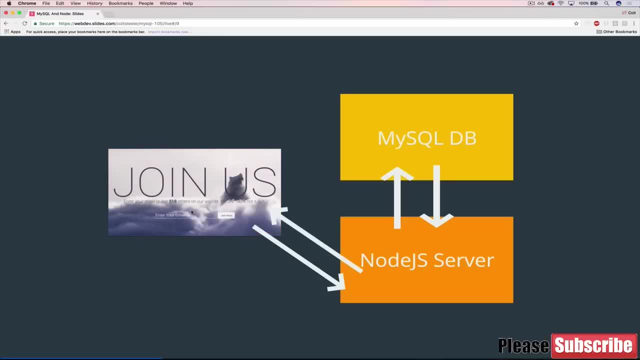 And I see the page. same thing, roughly the same thing happens when I enter my email and I click join. Now I'm sending my information, my email, to the node JS server With a message basically saying I want to add this, I'm signing up. 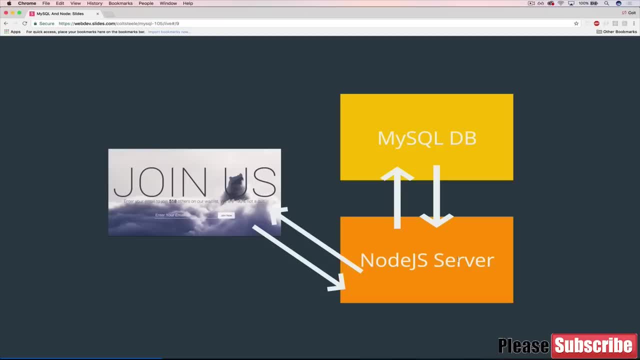 So then my server says, oh, this time this person is trying to sign up. They're not just asking for the homepage, They're trying to sign up. Okay, My SQL. I'd like to insert this user with with this email address: 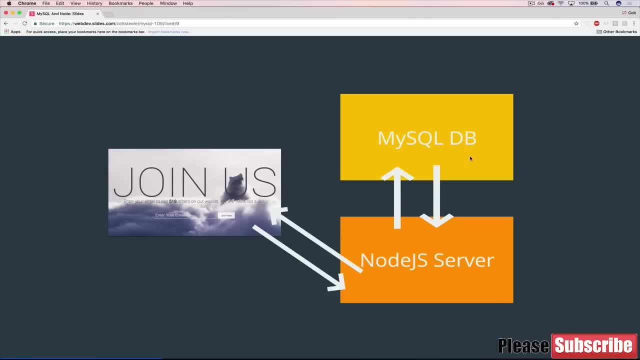 Then my SQL will say: that worked. or oh, we actually already have a user with that email, So we can't do that, or something else. Maybe there's an error that will be sent back. No JS figures out what to do. Do I send an error message? 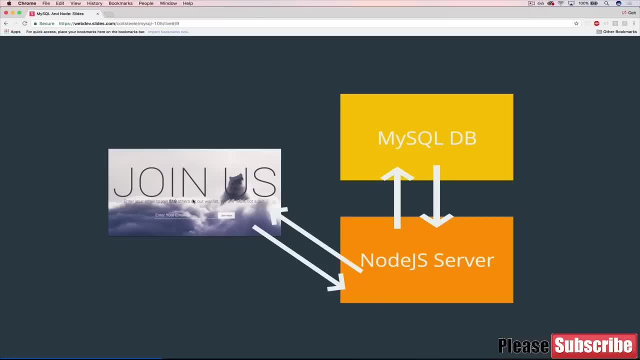 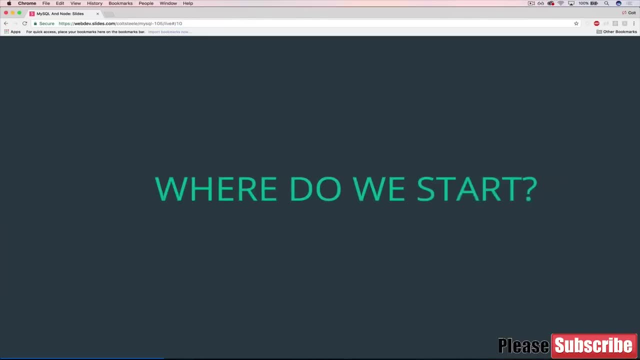 Or do I send a congratulations success message? Do I just take them back to the homepage and refresh it? That's, you know the decisions that are made here. So that's the basics. But then the next thing is: where do we start? 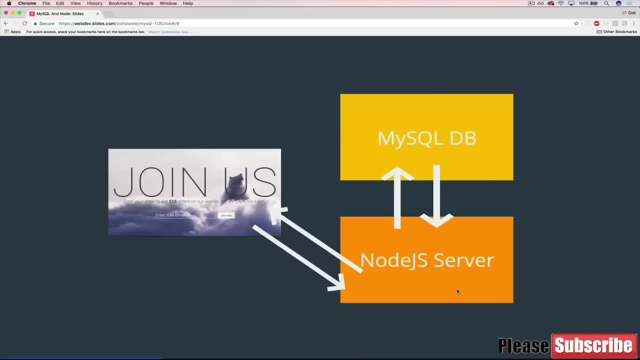 There's a lot of pieces here, right, We have to talk about node JS, installing that. We have to talk about how it communicates with my SQL. We have to talk about creating web apps and HTML and CSS and JavaScript- all of this stuff. 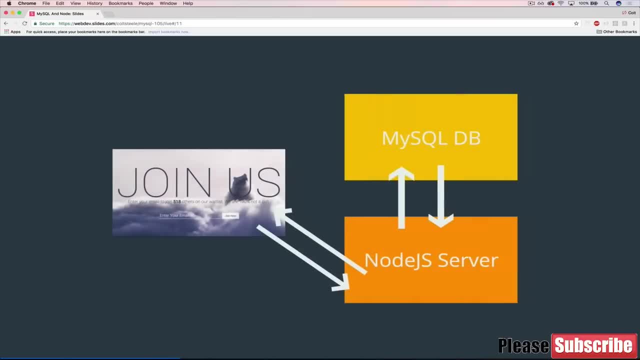 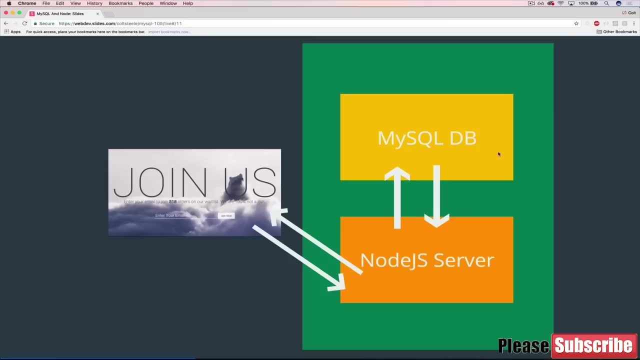 Um, there's a lot of moving pieces, So where do we start? Well, we're starting With this handy, dandy green box will draw your attention to the right side of the screen, which tells you we're starting basically with the relationship between node JS and my SQL. 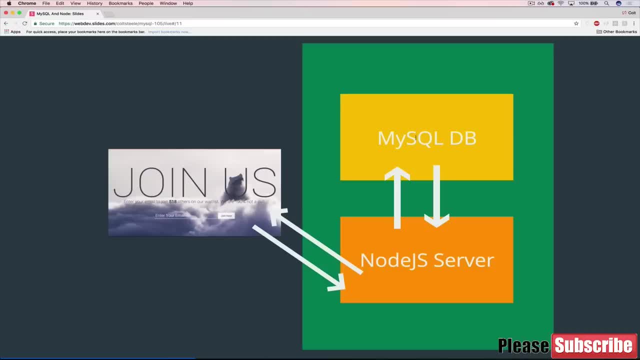 How do we talk from JavaScript to my SQL? So we're going to start with basic things like I want to select the current date from JavaScript or I want to insert a single user into my SQL. So no web app. this whole left side of the screen will be gone for the first part. 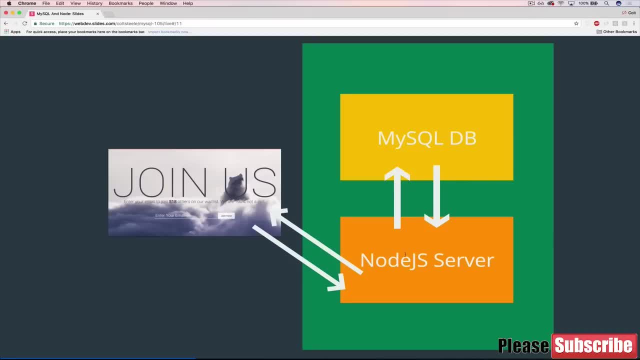 Uh, but then Once we have this relationship established- we figured out how to insert a user, We figured out how to select all users or select the count- Then we will then kind of expand into the web application and add in the logic for creating a web app. 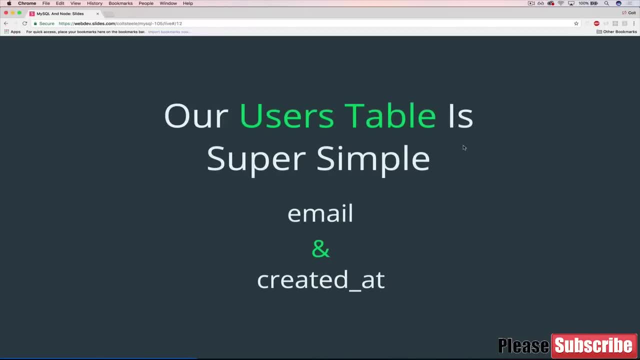 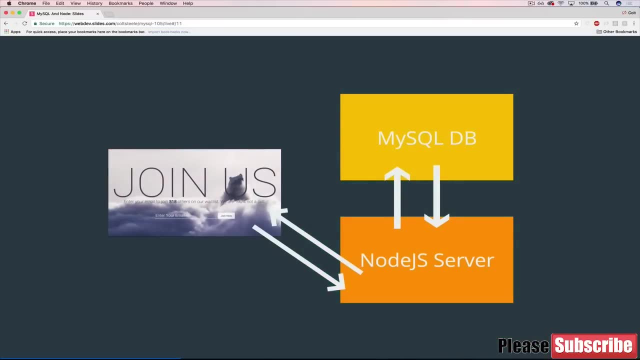 So that's our game plan. We're starting with this side, So the very last thing to discuss is what our table will look like. So for this web app, very simple, right, All that we need to store for every user. we'll just call it users. 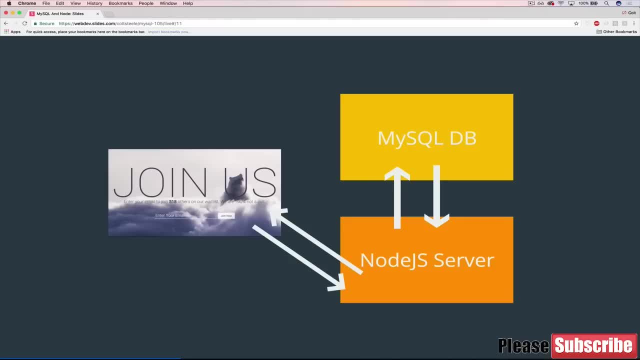 We could call it, you know, uh, Matt, email users, Yes, Starting email or specific email. So we don't just have to go with emails or interested people or whatever wait listers, But we'll go with users. 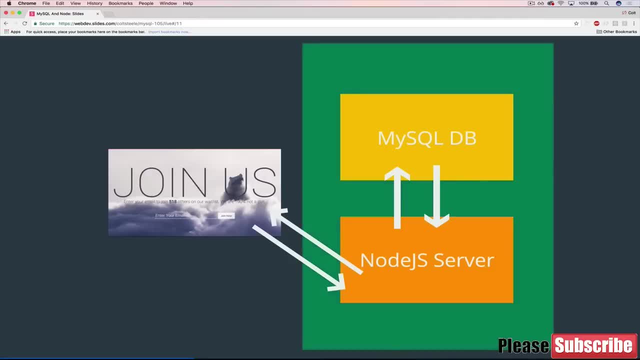 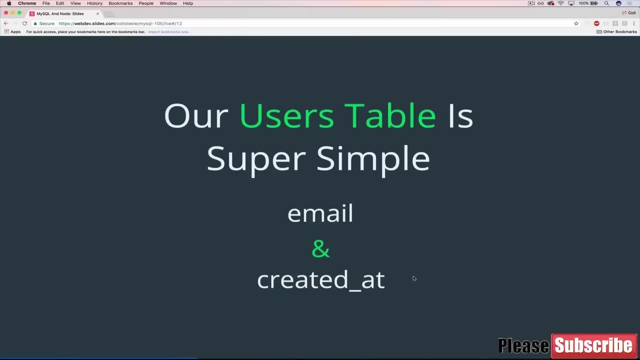 And all we need to store is their email address. right, That's a key thing. That's all they're entering, But it's also would be really useful to store a created ad, So we'd have a a timestamp for when that user was created, so that we could do things like figure out. 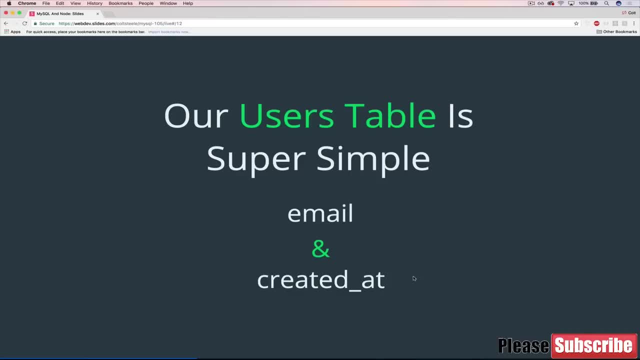 when most of our users signed up, or what day of the week most users are signing up, or just count how many users we've had, you know, this year compared to last year, and then when you get there, it's okay. 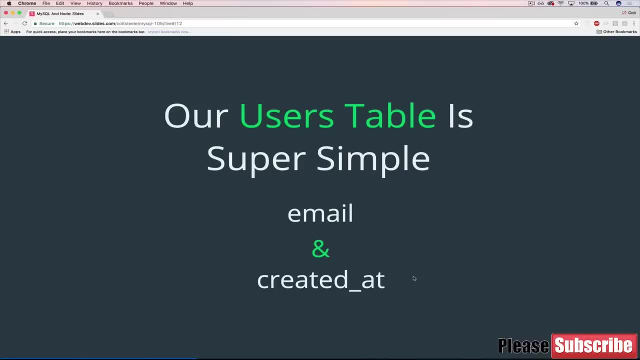 year compared to last year, So it's really nice to have created that. It's very simple as well. So those are the two fields we'll be working with, the two columns, and that's it, Nice and simple. And then the other thing to discuss is our game plan from here on out And our first goal. 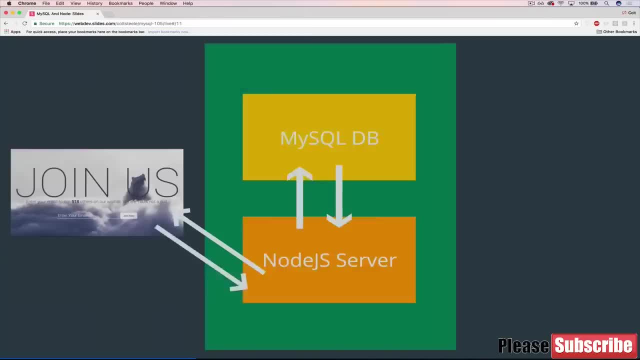 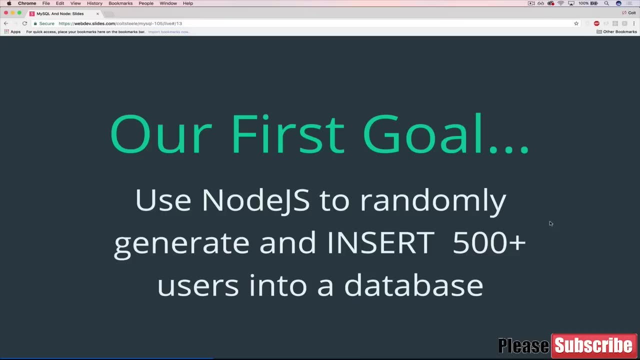 we talked about how we're only working with this side of the table or of this diagram. What we're going to work up to is using Nodejs to randomly generate and insert over 500 users into our database. So I had like 518 users in there. They all had unique emails. I did not 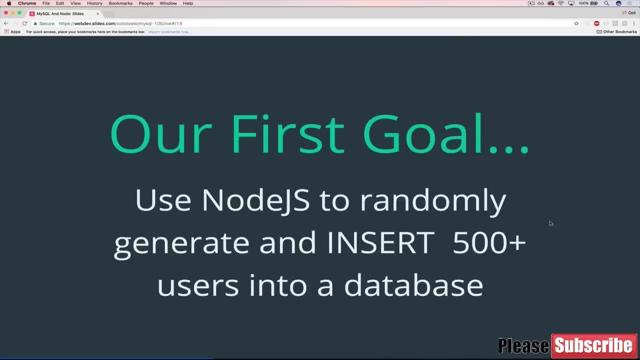 code those by hand. I used a tool that generates them for me And then I'm going to take that and insert them into our database. So basically shows you the power of using a language like Node, that we can very, very quickly generate data and not have to waste time getting 500 test users in. 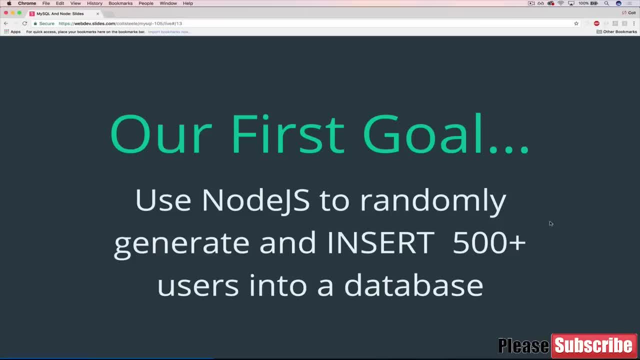 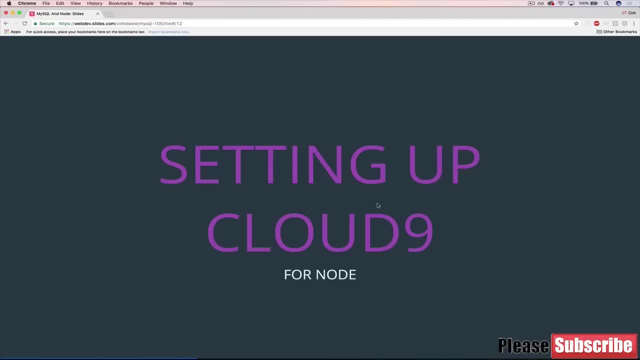 We've established we're working with Nodejs. Now we need to set up our environment so that we can do that. Fortunately, Cloud9 makes it really really easy. It's basically a single button, press, maybe two, and we have a Node environment ready to go. One thing before I do that: I do want. 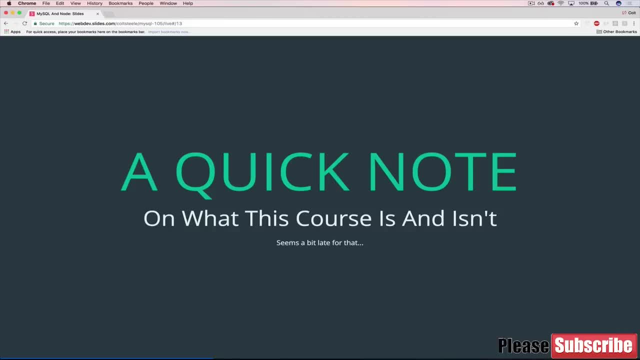 to talk a bit about what the course is and isn't. Yes, I know it seems like I'm leaving that a bit late, But really what I'm talking about is that this is not a Nodejs course. This is not going to be comprehensive. This is not going to teach you. you know a tenth of what you would want to. 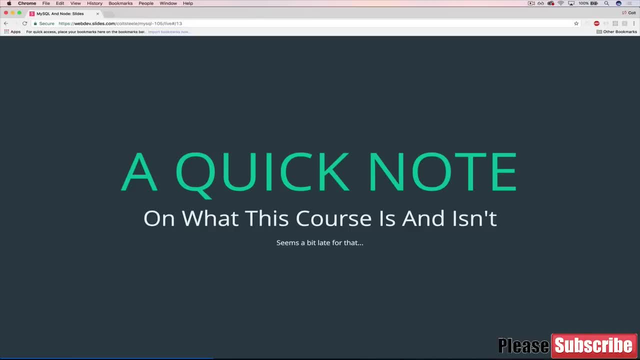 know about Nodejs if you wanted to be a Nodejs developer. This is not an HTML or CSS, or you know Bootstrap or whatever tools we use. It's not a course on those tools. They are helping us. They're serving a purpose, which is to make an app with MySQL. It's a MySQL course And we're. 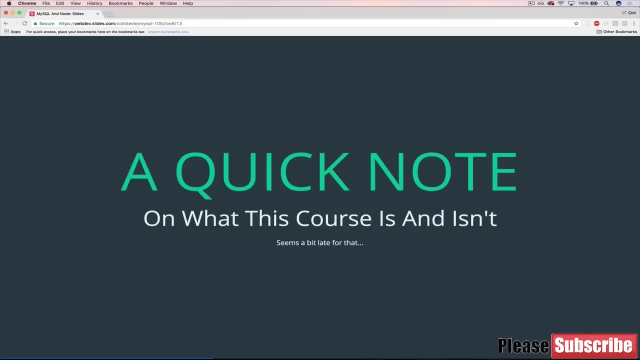 basically using those tools as needed. So I'll try and strike a balance as we go on here. I'm not going to just speed past and ignore. you know explaining what certain things are, just assume you know or assume that you don't care what you know a certain line of JavaScript does. 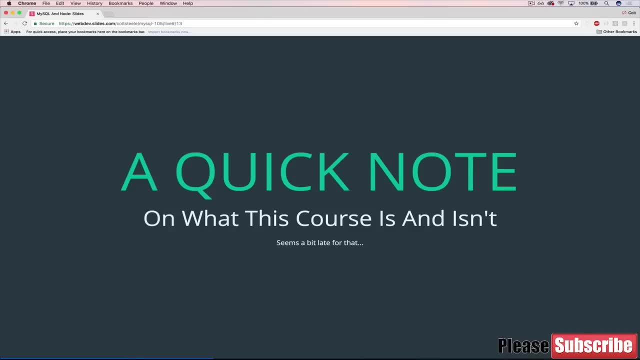 or what a line of CSS does. But I'm also not going to take the time to explain every single line to have you know, challenging CSS and HTML and Nodejs exercises and so on, We're still going to have exercises around MySQL. So I just want to throw that out there just to set your expectations. 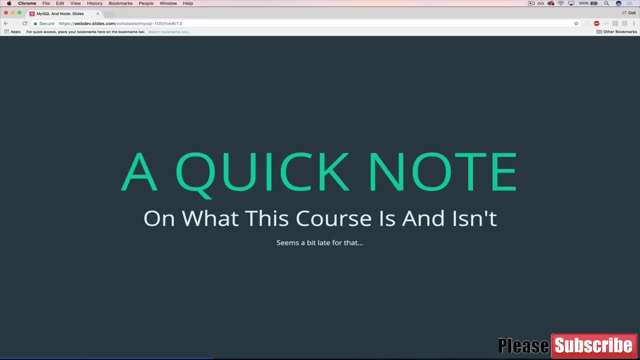 And also, if there is a chance that you want a full course on those technologies. I have a 45 plus hour course on those tools. So I'm going to take a moment and I'm going to take a moment and I'm going to show you the full course on those technologies that you can check out, But you 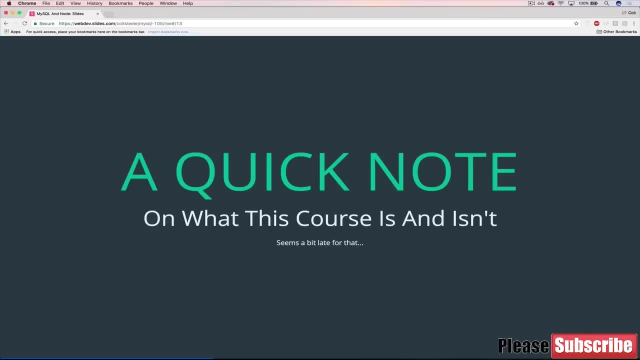 don't need that course to get through this. That's kind of the point. I'm going to show you enough, but I'm not going to spend 10 hours talking about Node Okay. so with that said, let's hop over to. 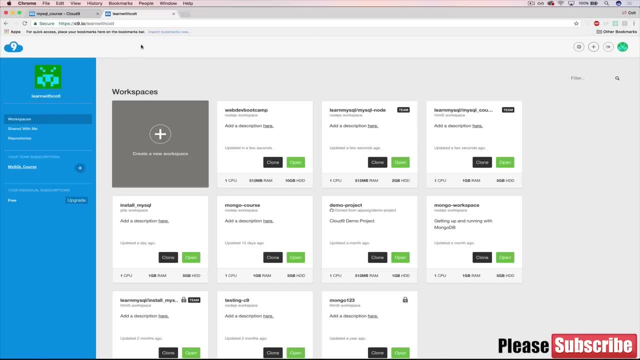 Cloud9. And we're going to go to our main kind of dashboard, So not inside of the editor, that's inside the Cloud9 environment, but we're going to go to our dashboard And you can get there, but it's going to see nineio signing in if you're not signed in. 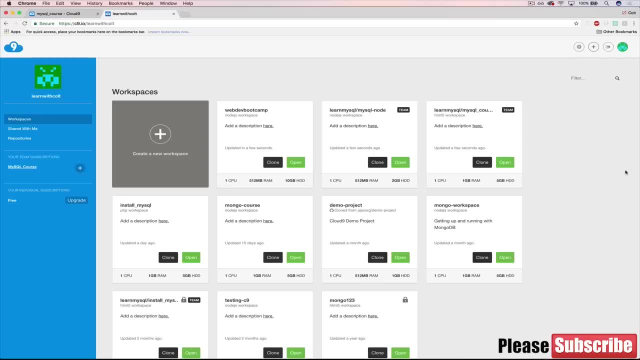 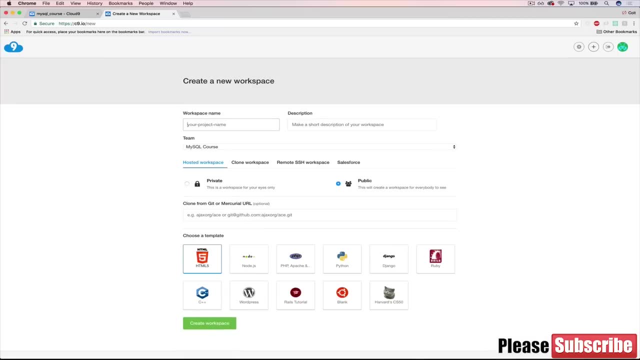 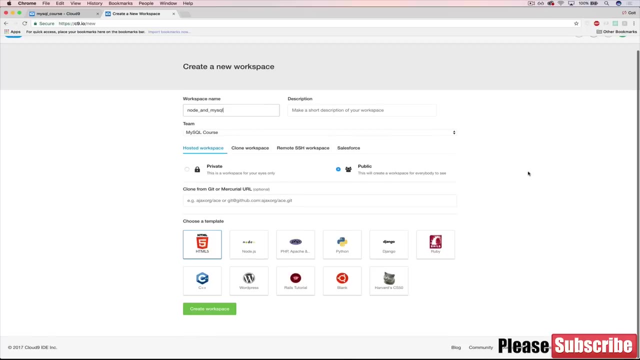 here Now I have a bunch more than you probably have, unless you've been playing around, but all that you need to do is click on create a new workspace And we'll call it whatever you want. I'll call this node and mysql, You can call it whatever you'd like, And then what we're going. 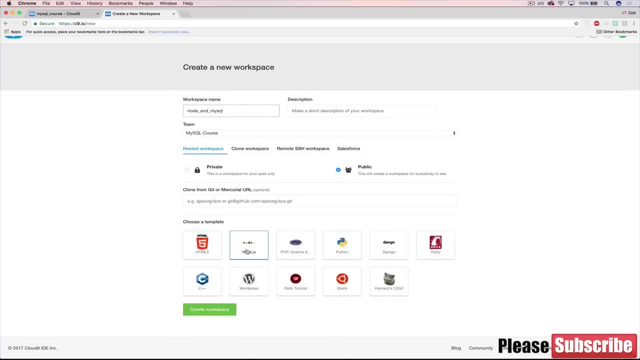 to do is down here- this is the important part- click node. So we could get away with any of these. We could install Nodejs ourselves. It's not actually terribly difficult If you want to install it yourself on your own machine. there are great instructions online. 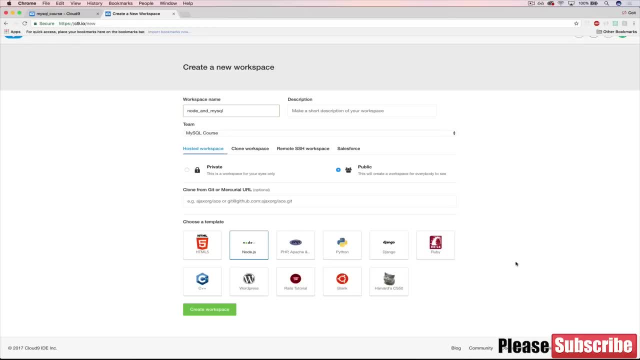 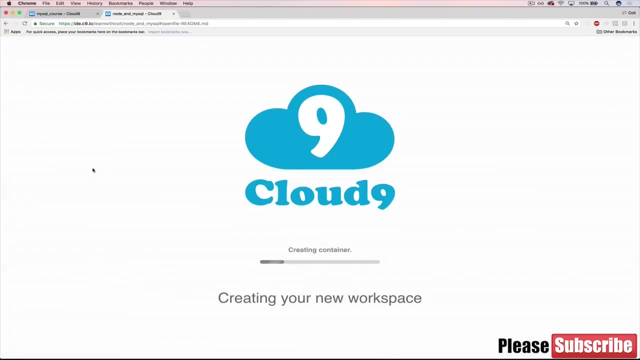 Just go to the Nodejs website. You basically just download a package, But we're going to be doing this using Cloud9. It's going to make it very easy for all of us to be on the same page. And that's it, Nodejs. give it a name, Create it. It'll take a little bit. I'll use the magic of editing to fast. 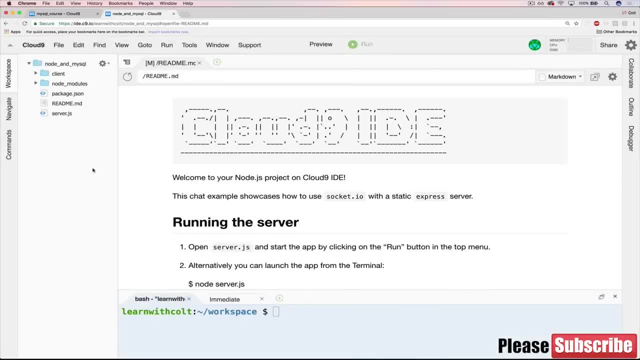 forward through this And we're back And this is what we see. So there's a couple things. One, we have a new environment. None of our old files are here, None of our old databases, the books or whatever we've been. 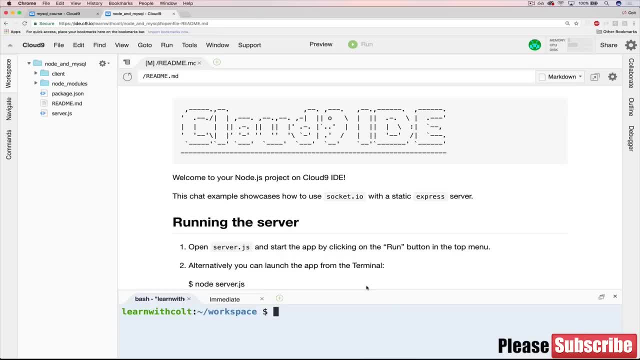 working with customers orders. that's not here, It's not gone. You would just have to go back to that environment. But, more importantly, we have Node installed here And we want to test that out to make sure. So what Cloud9 does is they actually give you kind of a starter app that we'll just 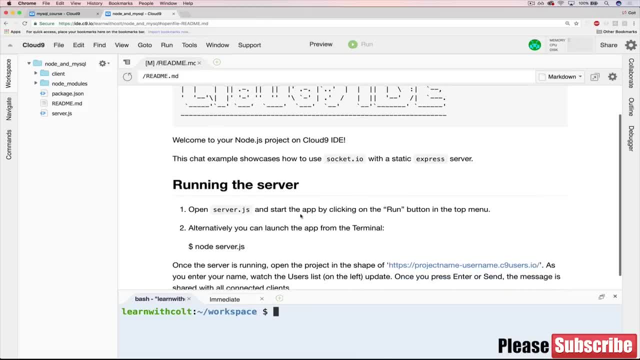 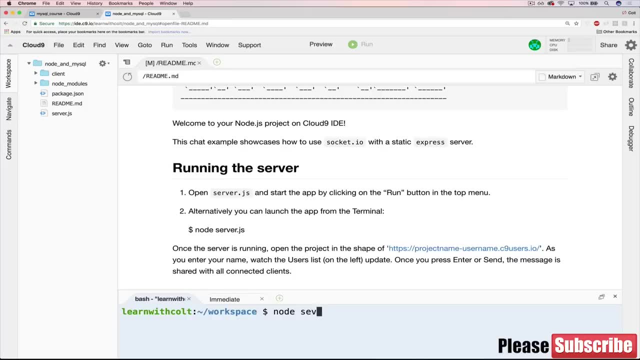 delete. But before we do that, we'll just make sure it works. So they have instructions. If you want to try it, all that we have to do is type node serverjs And actually, before I do that, ignore my ice maker. It's very noisy. If we just do ls, all right, we see, we have serverjs, Let's just 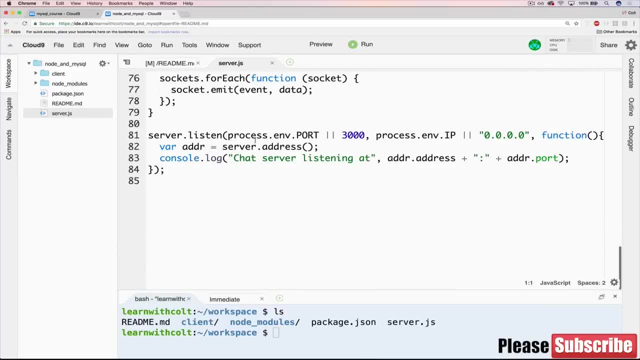 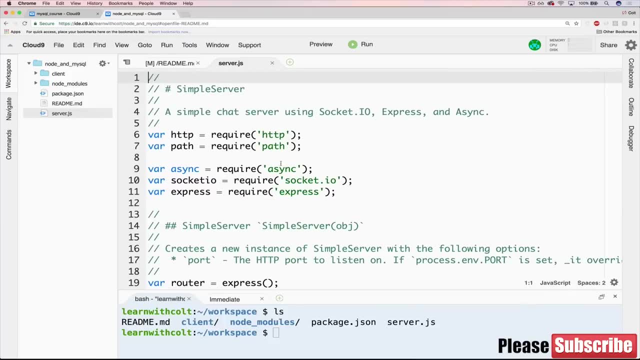 open it. There's code in here that we didn't write. We're going to get rid of all of it. And there's my fridge now. Boy, so noisy. Hopefully they're done now. So we've got all this code that we didn't write. 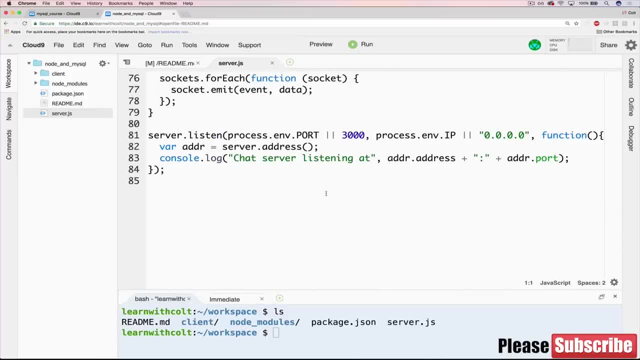 This is Node, This is JavaScript. We'll be getting to stuff like this. We're not going to make a chat app, That's what this is, But we'll be working on something similar. So now, if we do node serverjs and I hit: 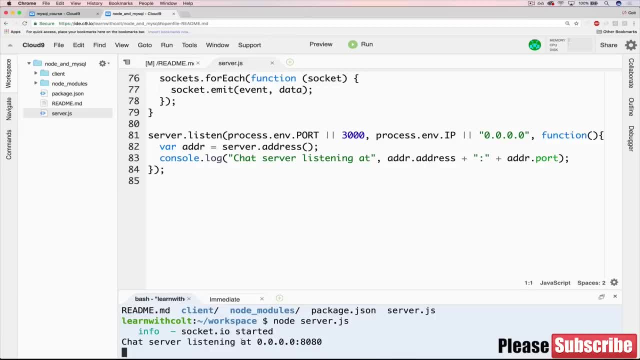 enter. we should get something like this Chat server listening at 0.0 blah, blah, blah, blah, blah, 80, 80.. Okay, So that's the first thing. If you get that, that means that Node is working. If you get. 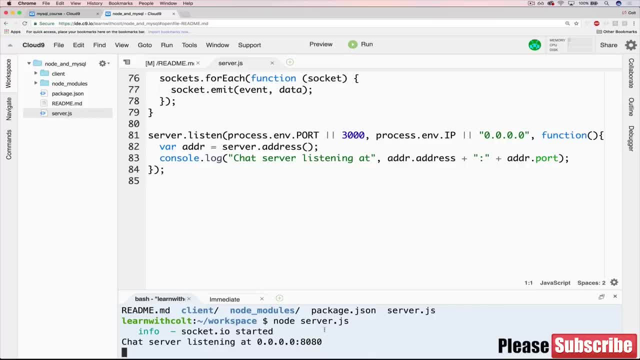 something like error command: not found Node, that means that Node is working. If you get something like that, that means that Node is not installed. And I highly doubt you would ever get that if you had created a new workspace and done this kind of the way that you're supposed to. But if you're 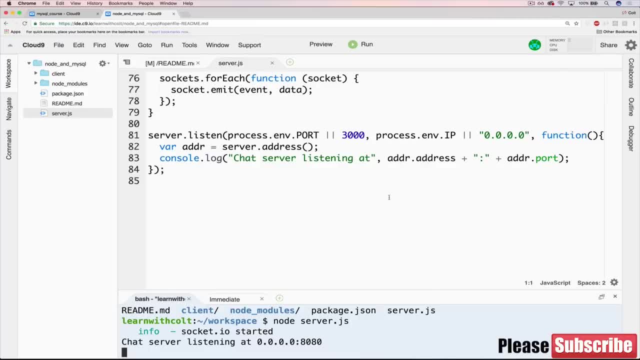 just working on your computer or you're working in a different Cloud9 workspace that isn't set up with Node and you try and type Node, then you'll get an error, And then the next thing to discuss is: okay, we have our app running, We started a server. Now how do we interact with the app? 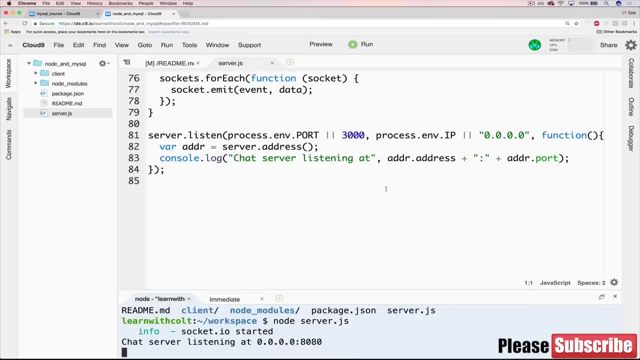 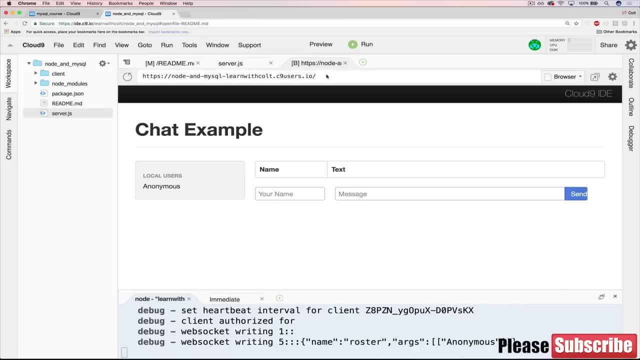 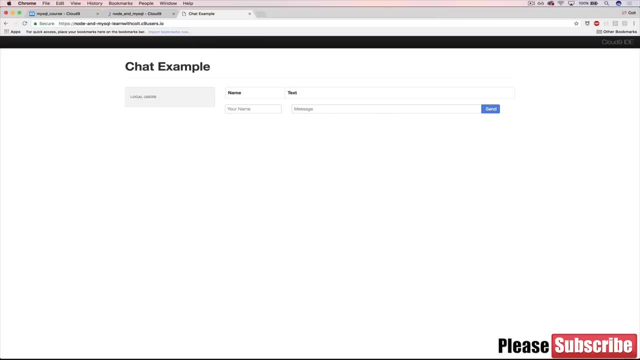 which is something we'll be doing. once we create our web app, We'll start it up and then we'll view it. You can actually click on this preview button, just go to preview running application and here it is, Or you can also just copy this URL. I like to keep it in a separate tab. 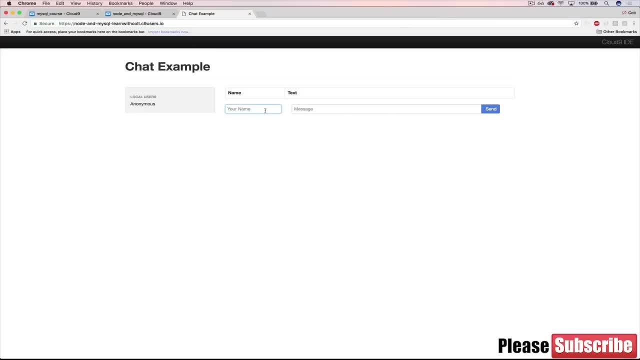 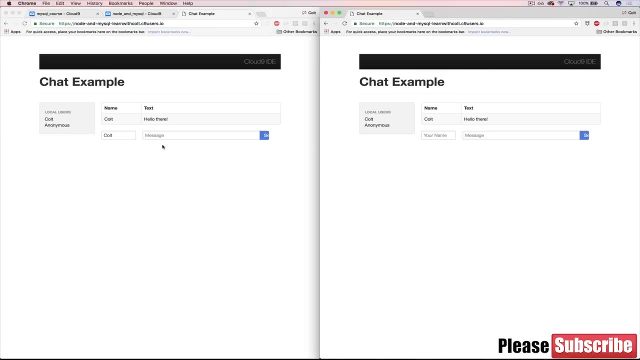 and just paste that in And we have a chat app now, If you wanted to. this isn't part of the course, this is not important, that you understand, but you can send it And I can do this in two windows. Now we have Colt and anonymous, so I can decide on a name. It's my cat And my cat says meow. 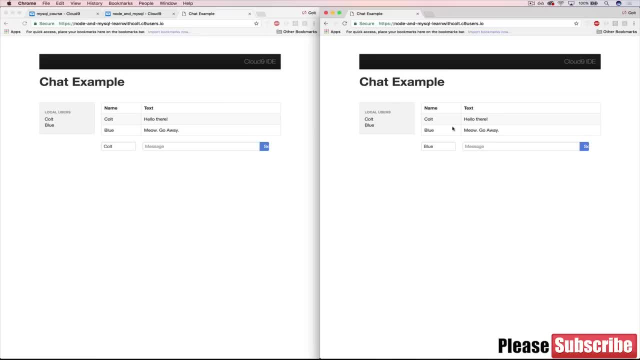 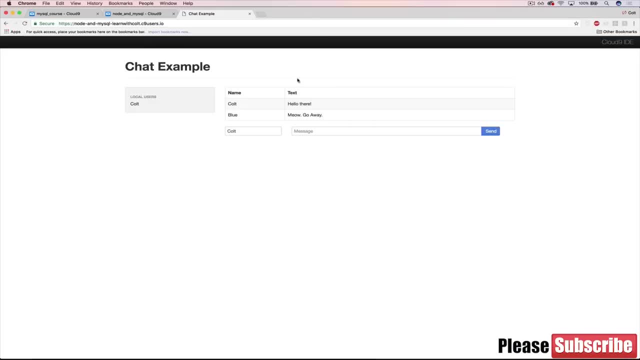 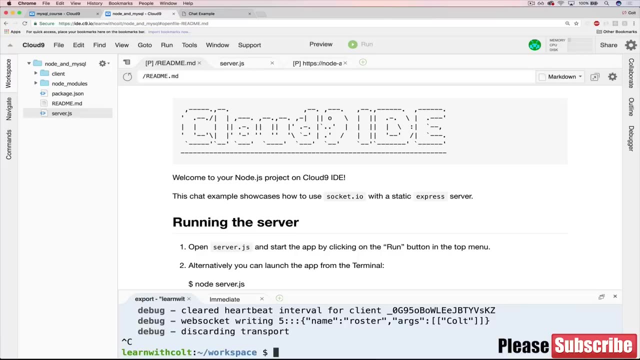 go away. send that. Anyways, you can see we have a chat app working. Here's a simple web app that we didn't create, but is running with Node, And that's important. Okay, so we can stop it using control C, just like we could stop the MySQL CLI, And that's where 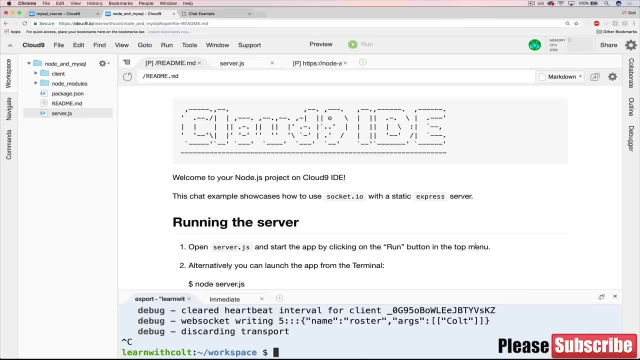 I'm going to end this video for now. Next we're going to do sort of a five minute crash course on Node, But for now what we talked about was creating the Node environment. We have this environment, And then we talked about how, if we have a server running, we can preview it by 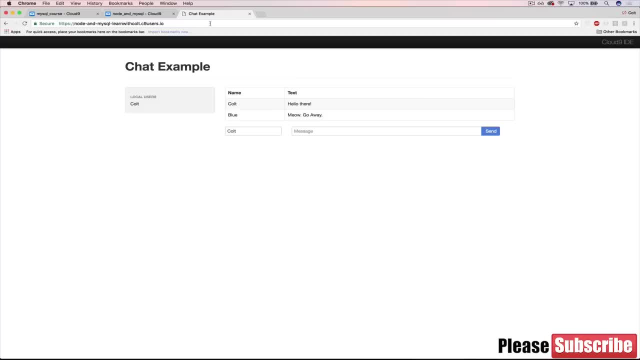 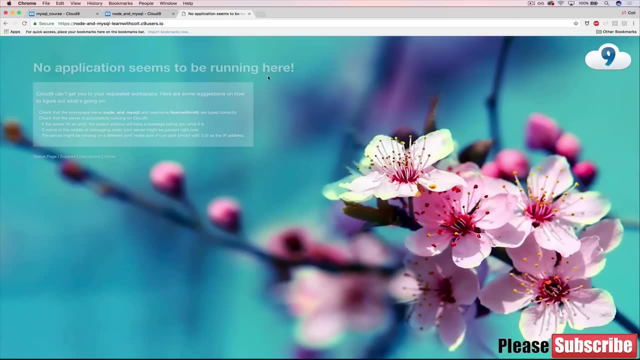 clicking on preview, or we can open it in a separate URL or in a separate tab or window. One thing to note: I stopped it, So if I try and refresh the page now, I get an error. There's no application running. Okay, so. 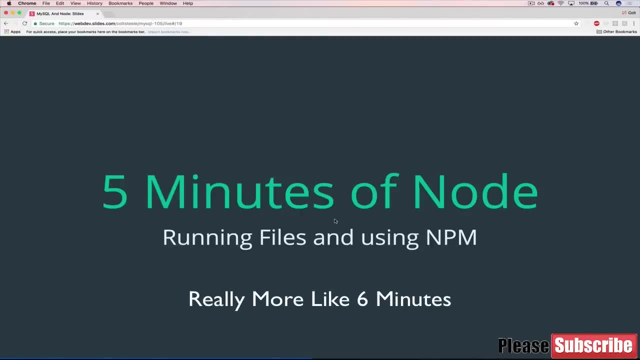 it's time for a five minute crash course of Node and JavaScript. Obviously, that's not enough time to even scratch the surface, But I'm just going to show you the basics of what you need to know for us to continue on with the course. Okay, so back over in Cloud9, we will delete everything. 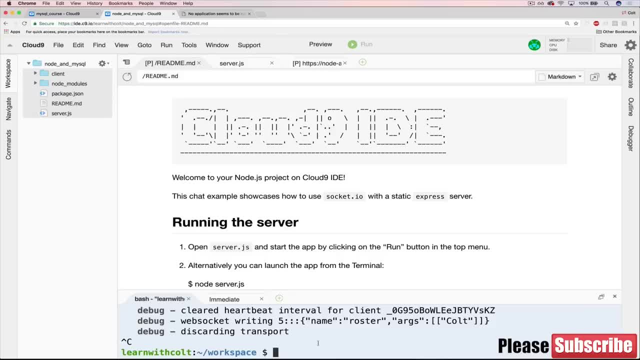 get rid of it. So you can do that. either, if you want to use a command line, you could do use RM and RM dash RF, Or just highlight what you need to delete, right click and where's that delete, And then we'll start. 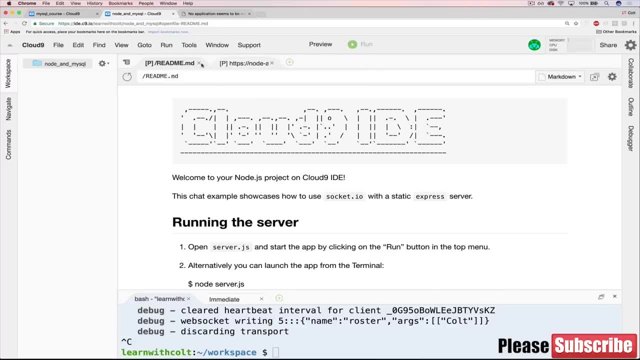 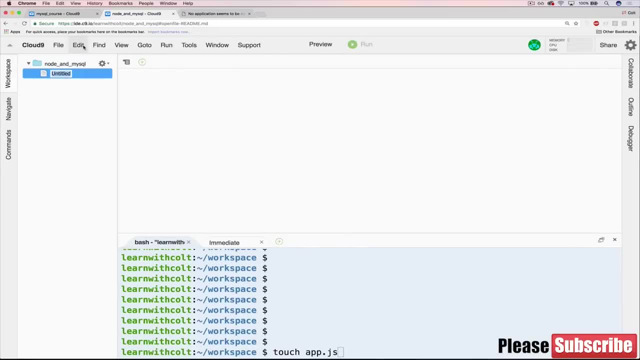 yes to all. We want to remove all of it And we're home free. now We can get rid of some of this stuff. Perfect, Make some space. I'll bring this up a bit. And now all that we're going to do is make our first JavaScript file. We can call it whatever we want. You can either. 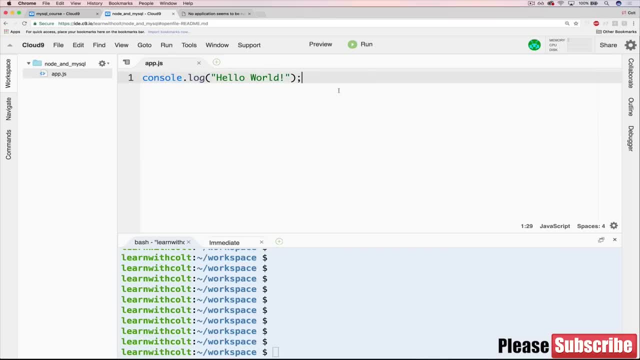 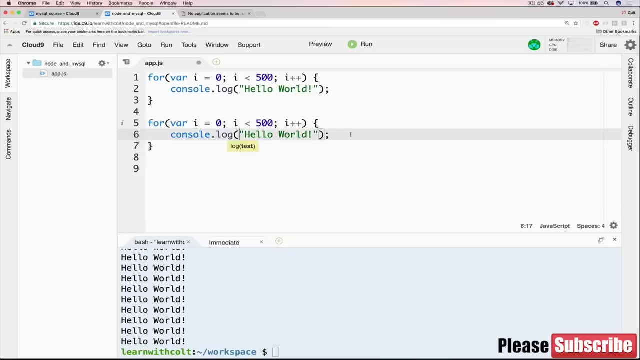 use touch appjs, or you don't have to call it appjs, or you can right click over here and click on new file. I'll do that one And I will call this. well, I'll do appjs. It's a standard name, Okay, And I won't recreate it down here. Now we'll open it up double. 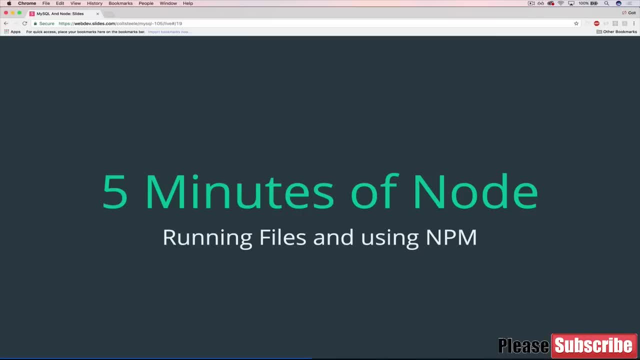 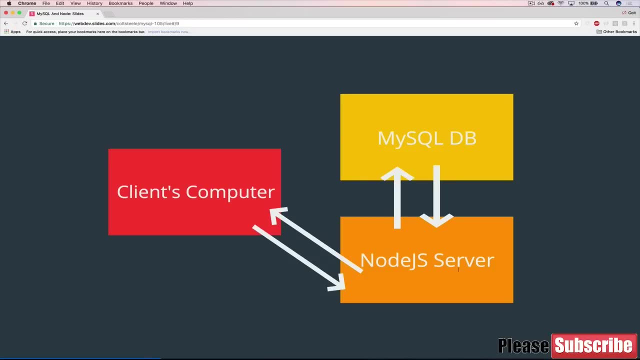 click and we'll add some JavaScript in here. So what I want to show you is this basic workflow with node that we kind of saw already. We type some code in a file, we save it and then we execute the file with the command node space. 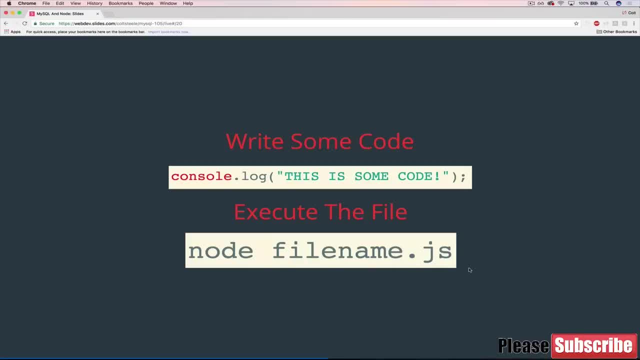 And then the name of the file. So it's very similar, at least in principle, to what we did with the SQL files, where we would save a SQL file ending in sql, put something in there, a query, then we would execute it using source and then some file name- sql- Same. 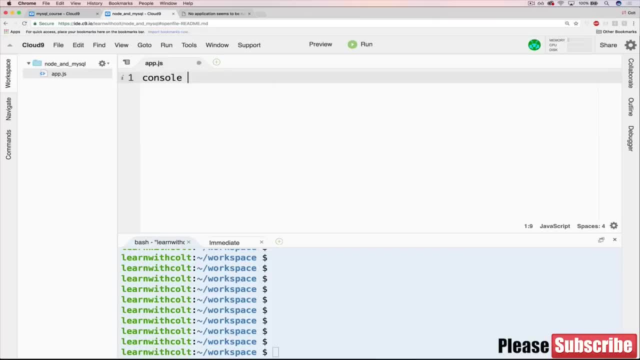 idea, So I'm going to show you some very simple code. There's something called- and again, if you know this stuff, feel free to skip it- something called consolelog, kind of the simplest possible command And what we can do in MySQL. it will just print something out So we can do our basic. 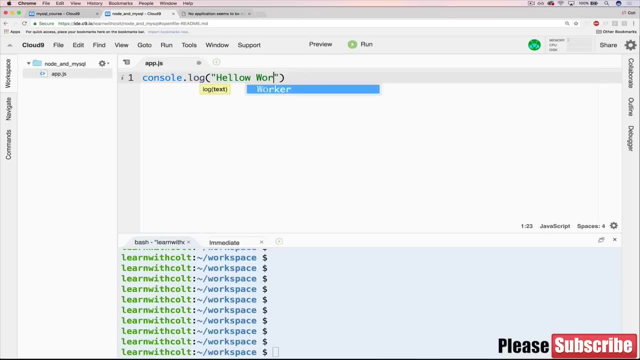 hello whoops, we don't need caps, hello world. and we'll put a semicolon there which should seem familiar from MySQL at least. And let's start with this, our first application, very basic And all we need to do to execute. 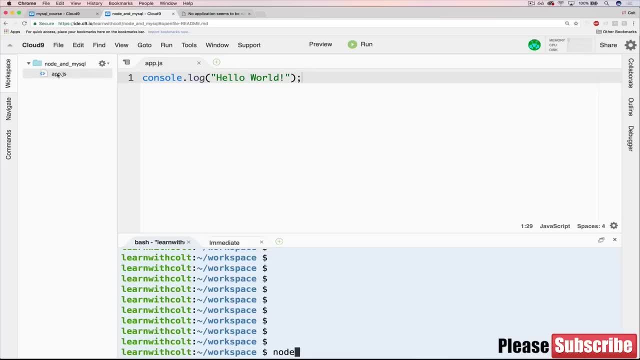 it is come down here and type node and the name of the file, which we called appjs, And it runs Silly but it works Okay. so that doesn't seem useful, of course, but it's something right And to see kind. 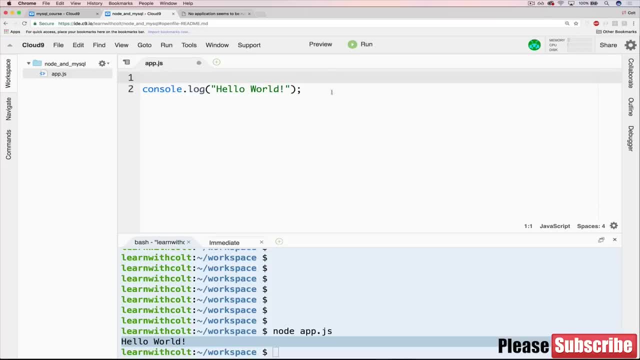 of why a programming language would be useful. let's at least do this 500 times Let's. maybe that's not useful, but we can at least see how it's helpful at doing something that we can't do on our own. So we can create a simple loop. We'll do less than 500.. 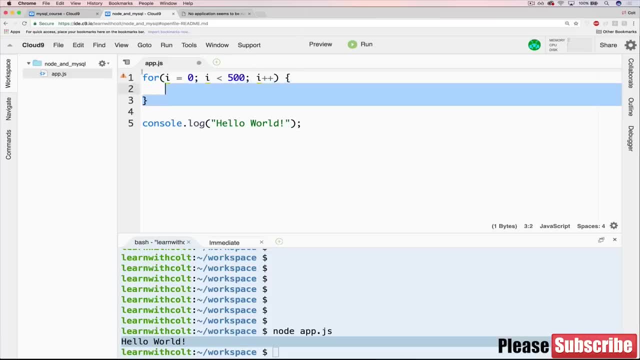 Now in my other courses. this is like an entire video- 5 or 10 minutes- with exercises, but I'm not going to spend time on that. What this here does is it says whatever's inside of here. repeat 500 times, Basically. 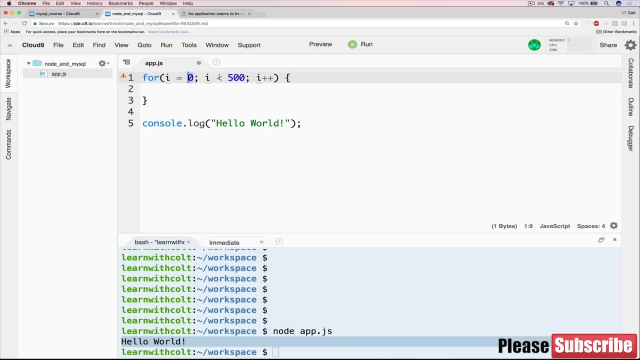 this is a counter saying: OK, we're starting at zero And every time through the loop we're going to add 1 to I, which is what this does here. So we go zero next time around 1,, 2,, 3.. Keep going while it's less than 500.. As soon as it hits 1, that is a 100. That's. 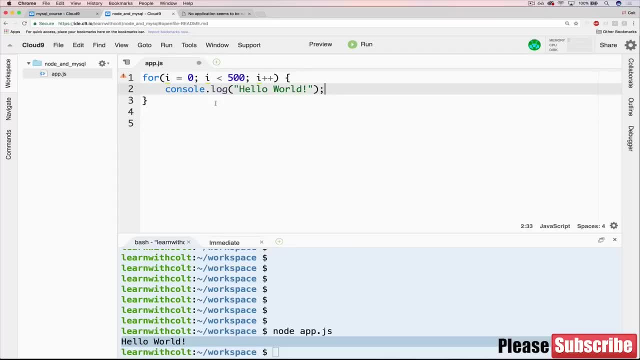 As soon as it hits 500, we're done. Okay. so if I just put that in there, whatever is in these brackets here will happen 500 times. Let's do it now. One thing I could add that I probably should is this: var keyword. 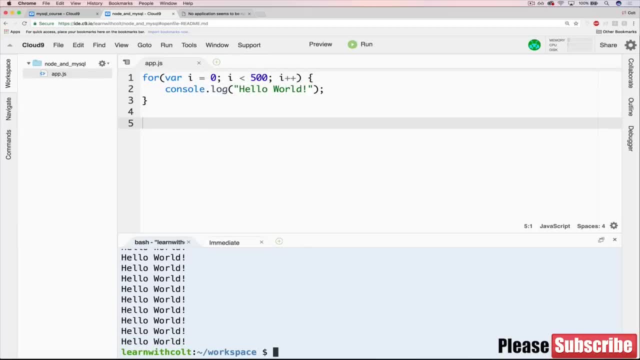 It's just, don't worry about it, but it's important to have it there. Now, if I run it and I scroll up, you can see we get hundreds of hello worlds- Well, 500.. So imagine you might be wondering why do you care? 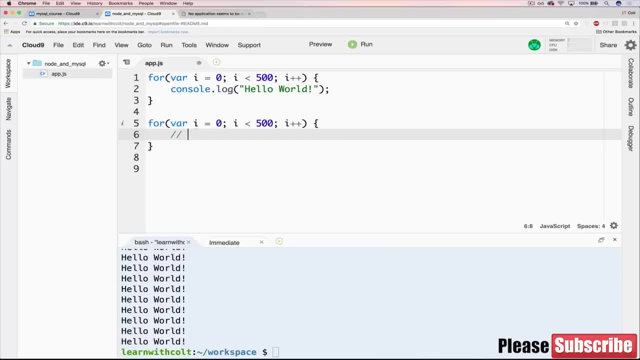 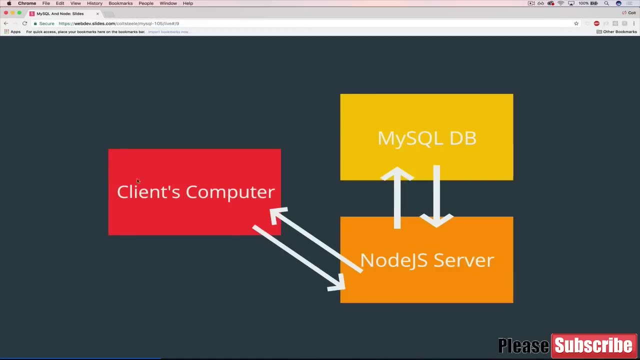 Well, imagine, instead of consolelog, what if we had insert a new user into the database? That would be a fantastic way to quickly seed a database with a bunch of data. Remember how we had to do this obnoxious copy and paste? So I would give you a file you would copy and paste, like for the movies, data and reviews. 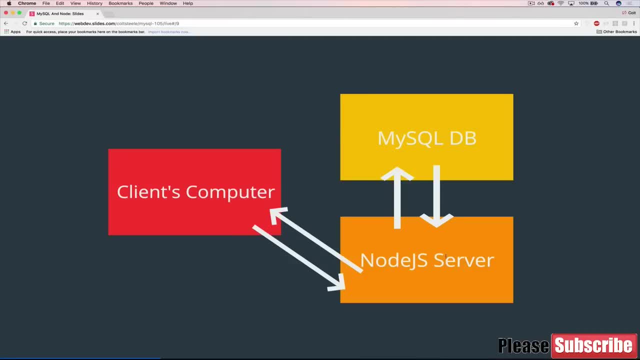 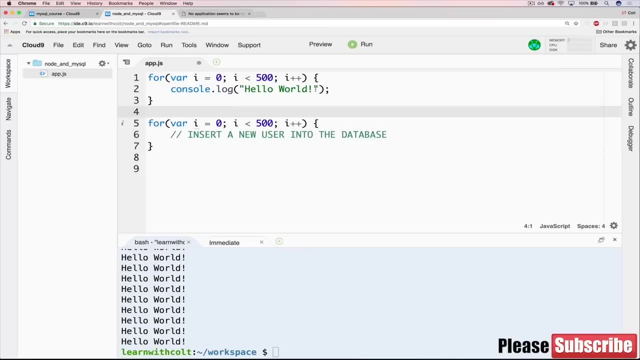 there was these big files. you had to copy and paste it in. It's an awful way of getting sample data. Well, we can use JavaScript to create data for us. So just a couple other things that I'll show you. We can do math and basic things like 5 plus 5, and I won't do this 500 times. 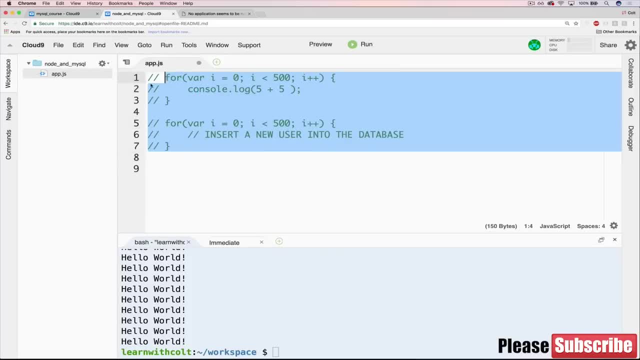 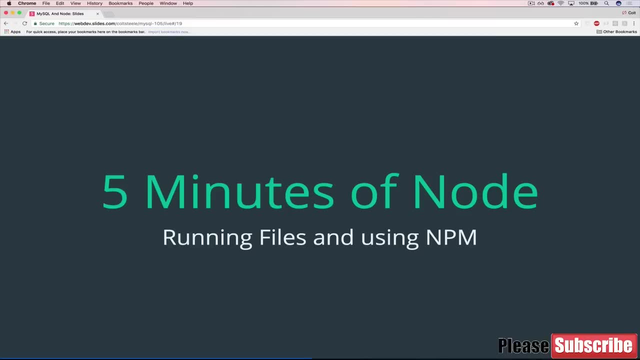 We can comment things out, selecting them and doing command slash so that won't run anymore. So now I'm only running 5 plus 5.. You can see we get 10.. One other thing to address is what is Node, if you're not familiar with it. 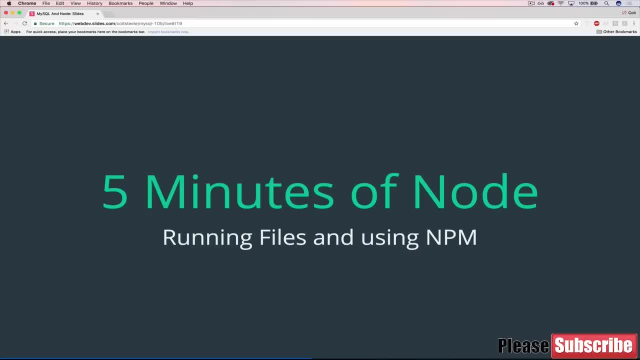 And that's actually a pretty common question. There's a bit of confusion about Nodejs, which is what it's called, and regular JavaScript and what the difference is. Basically, JavaScript is a programming language. It was created first. It's been around for a while. 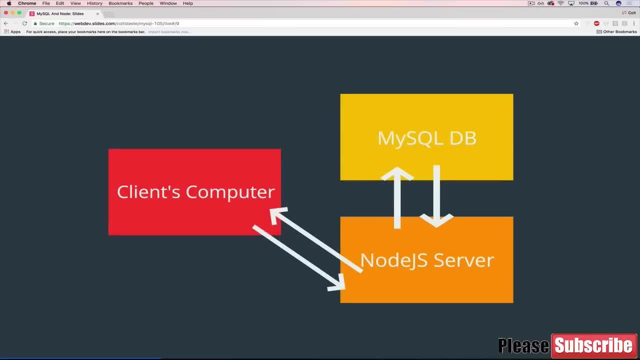 And it's existed as a language that you can use on the client side. So what that means is that back on this diagram there's a line right here- Not right now, but imagine a line. This is the client side- So I could write JavaScript code that did things over on someone's like on my computer. 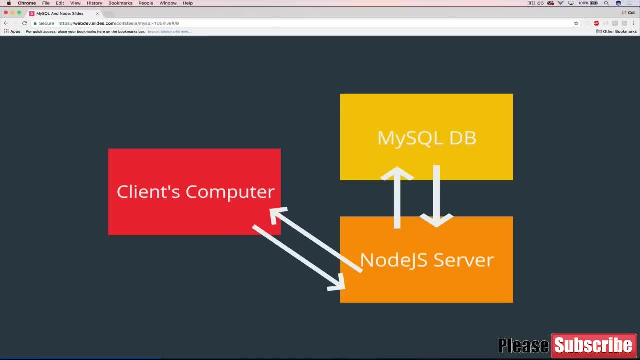 You could write code that would animate something or make a game or just add some pretty effects. That's not to say that it's not powerful, But traditionally it was used kind of to decorate pages, if you will, And it had nothing to do with databases. 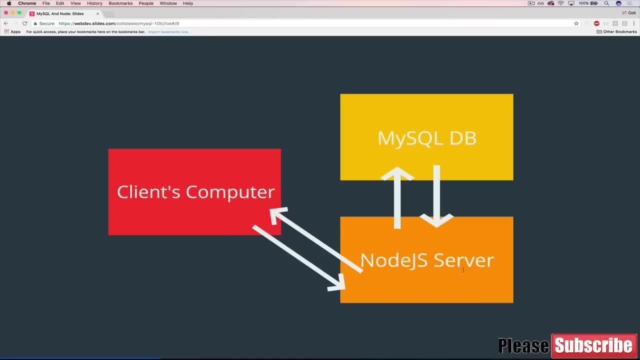 It had nothing to do with servers. You would use another language over here, like PHP, And you would use JavaScript on the client side of the front end. But then Node came around about five years ago now, And what it is is an implementation of JavaScript written so that you can use it on the back end. 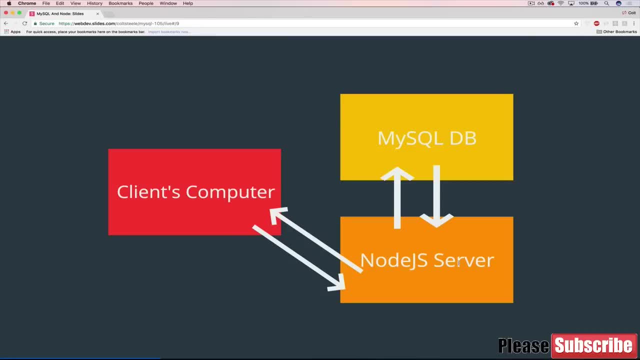 So that you can do things like this. You can create code, You can create a server with JavaScript instead of having to do it with Ruby or PHP, And it can talk to a database like any other server-side language. So, to summarize, that Node is JavaScript. 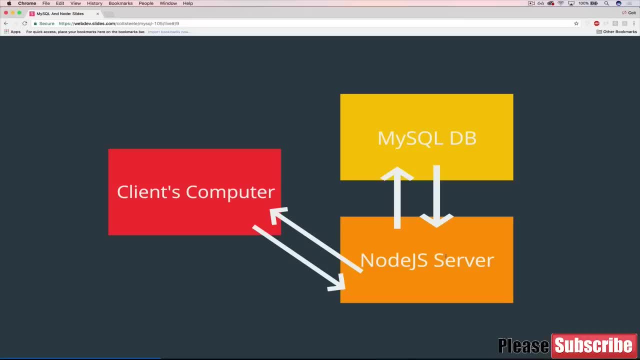 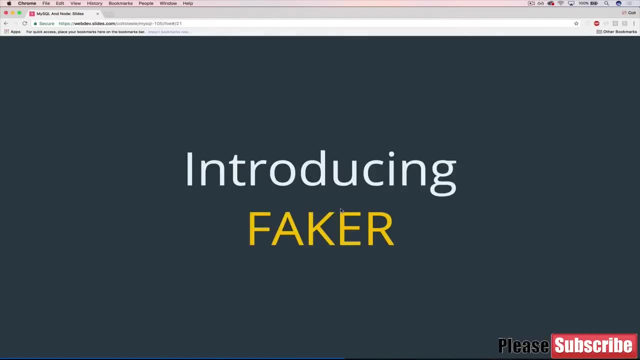 It uses basically the exact same syntax, But you can use it on the back end, which is what we'll be doing in this course. So I know that was a very brief introduction to two lines of Node and of JavaScript, But we're now moving on to more important things. 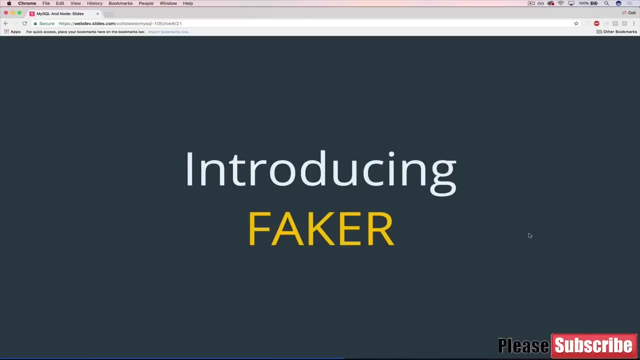 Things that are relevant to MySQL, And the first thing we'll do is talk about a package called FAKER. So the first question you might have is: what is a package? And basically Node comes with thousands and thousands of libraries. You might have heard them called or packages or modules. 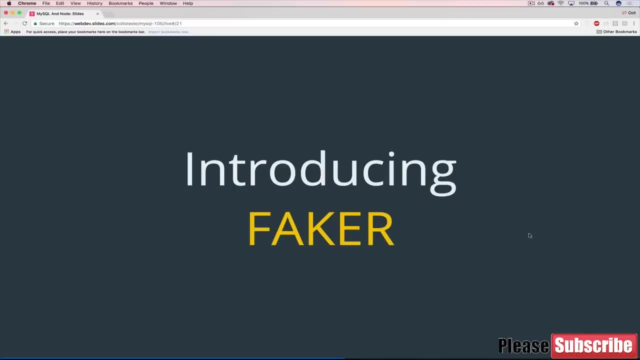 Code that other people have written that we can include inside of our application. really simply, All I have to do is say: install FAKER, which is the package we're going to use, But we'll use another package later called EXPRESS. 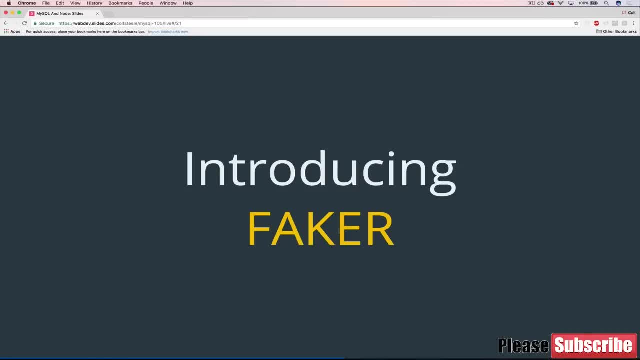 Or we'll use one called MySQL, And all I have to say is install MySQL, Install FAKER, And there are thousands of them out there. like I said, And that's one of the biggest strengths of Node is that it has a huge library of all these packages. 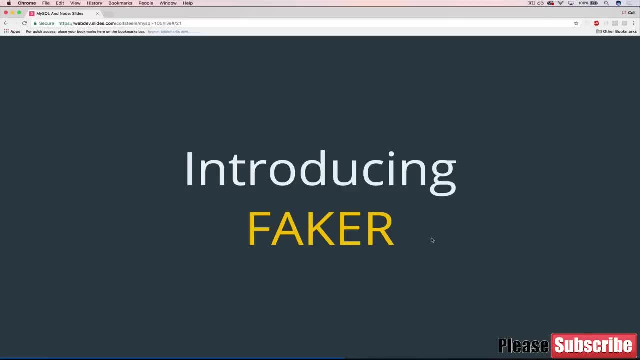 So that you don't have to do everything yourself. You can go and get some help by including somebody else's package. So the way we do it is through something called NPM- Node Package Manager- And to install FAKER, which, don't worry, I'll explain what FAKER is. 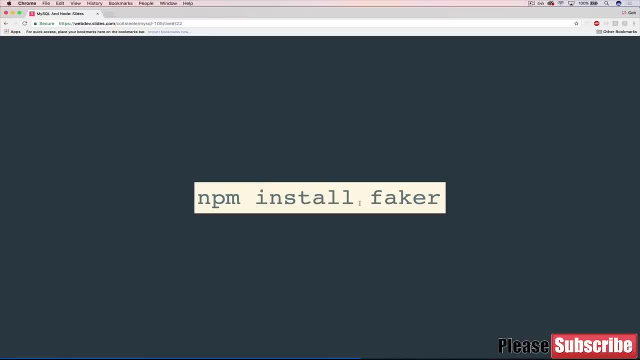 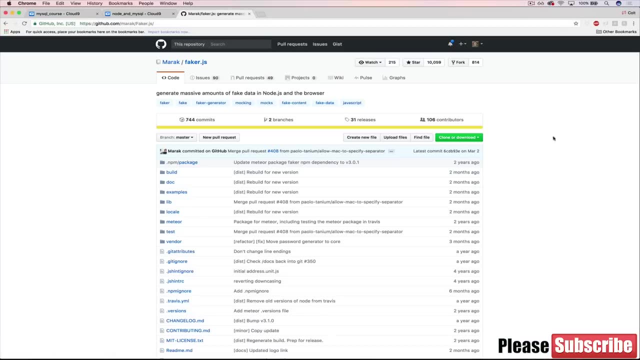 This is all we have to type Into our terminal: NPM- install FAKER. But before we go there, let me show you what FAKER is. So FAKER is a package that there's a bunch of different versions of it. 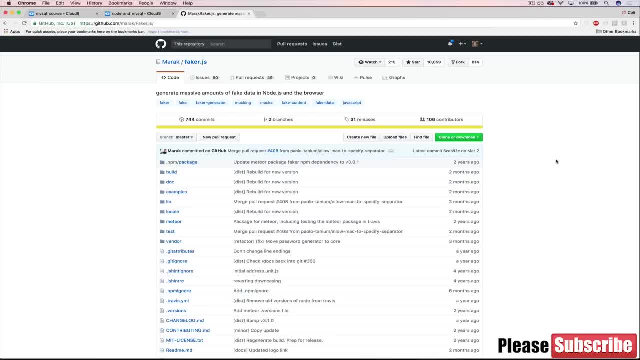 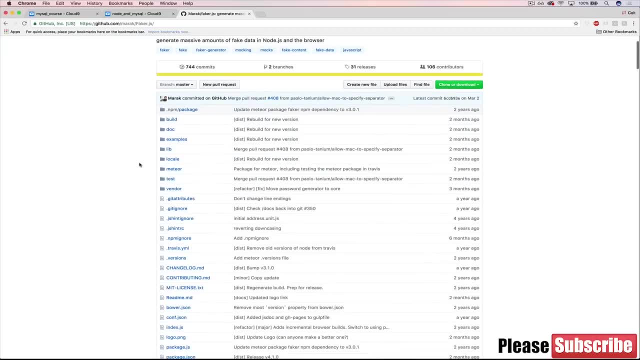 There's. I think the original one was for Ruby. I'm not positive, But there's FAKER kind of implementations for other languages, including JavaScript. And what it does is it really helps us? it streamlines the process of generating fake data. 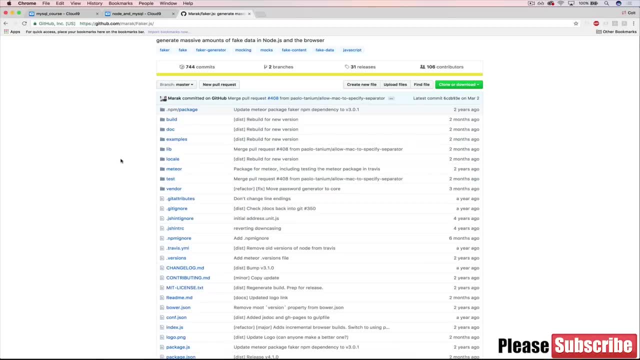 So we're going to use it Because we want to start off with a bunch of fake data in our database. I don't know if you noticed. I had 518, 519 users in my database. I did not enter those manually. 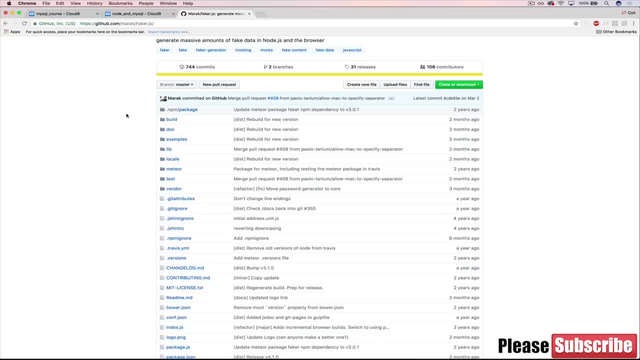 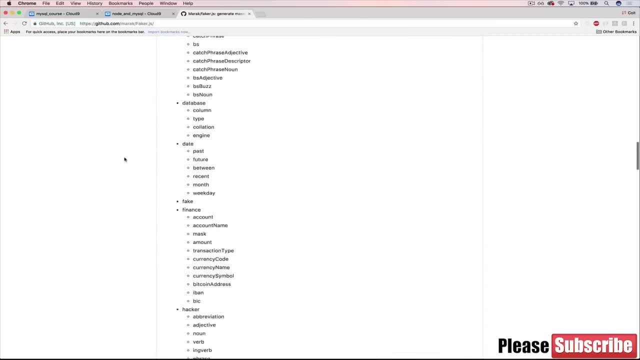 And they are. they're all unique. They have a different unique email address. I did not generate those myself, So we're going to use FAKER to do that. So FAKER is very simple. I can say things like FAKERaddresscounty. 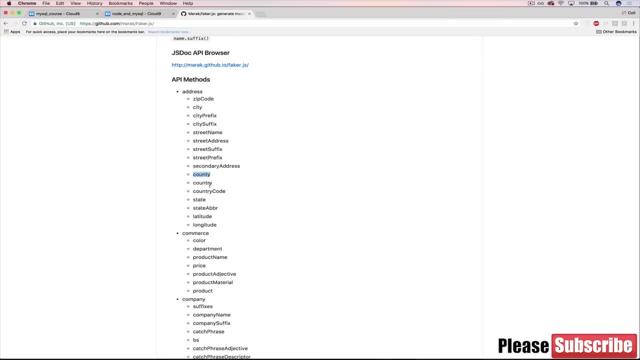 And it will give me a random county name, And it has hundreds of them. Or I could say FAKERaddresscounty, Or I could say FAKERnamejobDescriptor, And it will give me a random job descriptor. So there's tons of things in here. 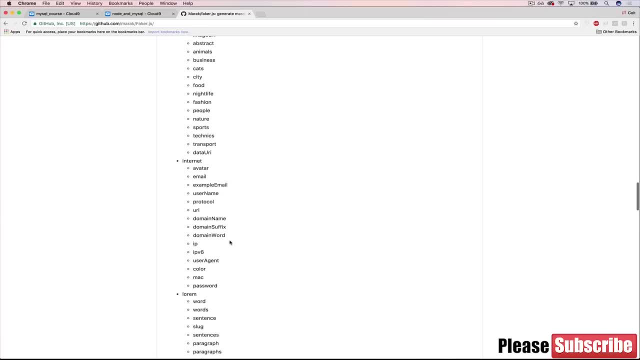 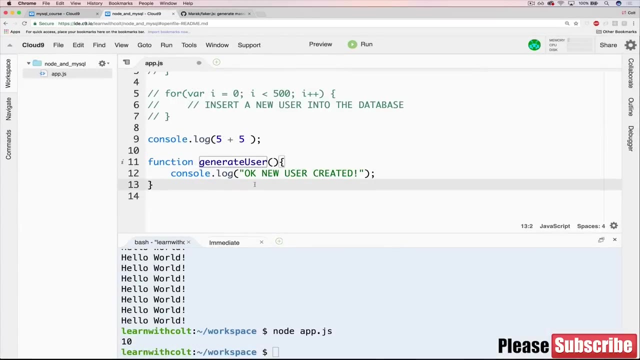 Phone numbers, random numbers, file names, colors, avatars, emails, usernames, domains, passwords- So many things that we could pick from Credit card, fake credit card numbers, account numbers. You get it, hopefully So, back in Cloud9. now what I'm going to do is actually empty this file entirely. 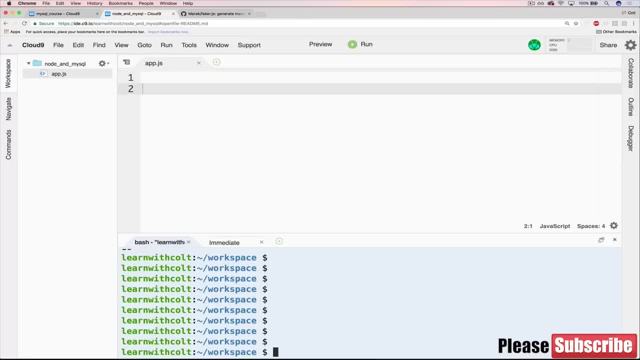 Appjs. You can make a new file if you'd like, And now I'm going to install FAKER so we can use it. So this video- I probably could have done a better job explaining this- is about two things. One, FAKER, but on a higher level, packages in general and how you use them. 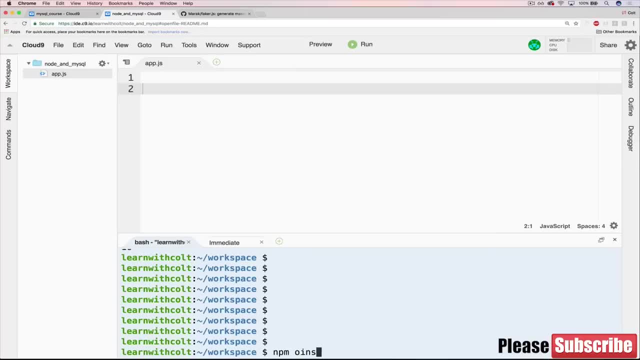 So this is the workflow for using a package. We type npm install name of the package and hit enter And it will take a second And that on its own installs a package. You'll notice I have a new folder here called node modules inside. 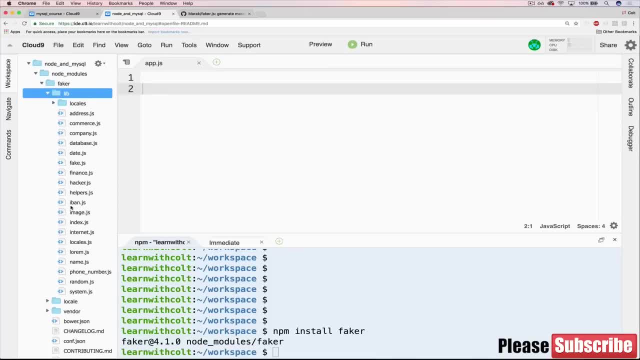 There's all the FAKER code, all this stuff. So all that is here now. I just had to type a single line. It's pretty awesome. Now in my Appjs I can't just start using it immediately, I can't just say FAKERemail or something. 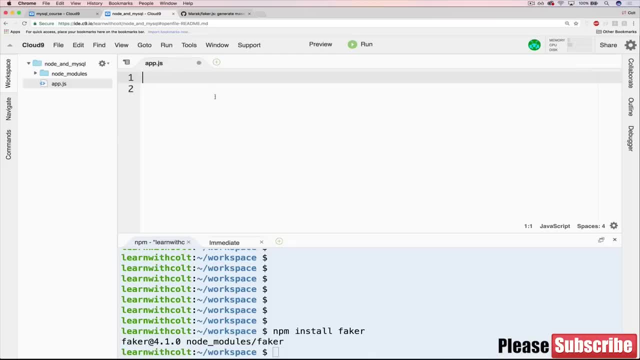 I first have to tell this file I want to use FAKER. I have to include it or import it, And it's very easy. I'm just going to say: var FAKER equals require FAKER. So this right here is a variable. 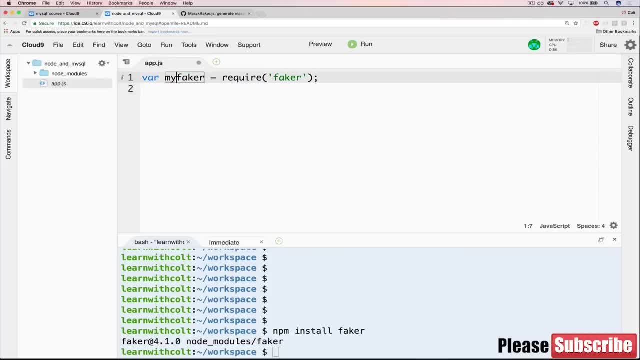 I can call this anything. I can say my FAKER. I'm going to call it FAKER standard And this is the part that I can't change. This has to be FAKER. So this is going to go find a package that I've installed in node modules with the name FAKER. 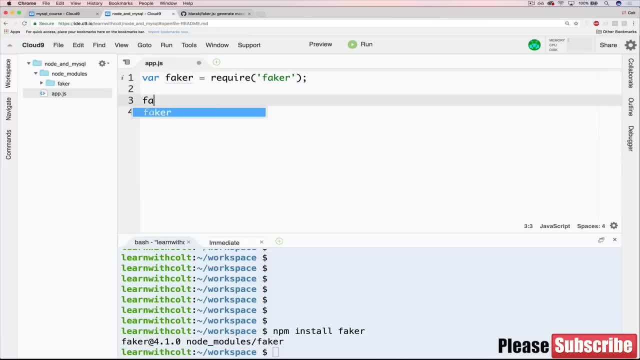 And then save it into this variable. So now, whenever I use the word FAKER referring to this variable, I actually am referring to the package, So then we can do things with it. So we could do something like this: FAKERinternetemail. 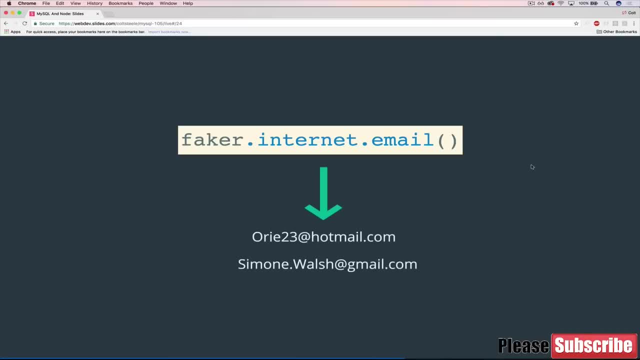 And that will generate things like this Or this Or this Ori 23.. Simone Walsh Aubrey. underscore dot tree Numbers. We've got Hotmail and Gmail and Yahoo, So this would be a pain if we were doing this ourselves to come up with 500 individual emails. 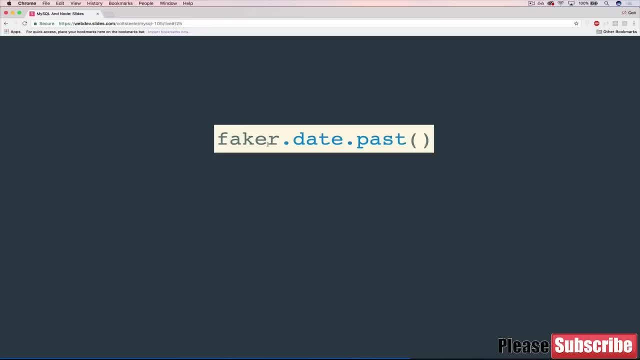 And the other thing I'll show you Is we're going to use it for dates, So I'll be able to say FAKER dot date And- this is important- Dot past. So we don't want to have any future dates. Basically, we want to start with 500 users in our database who have signed up at some point in the past. 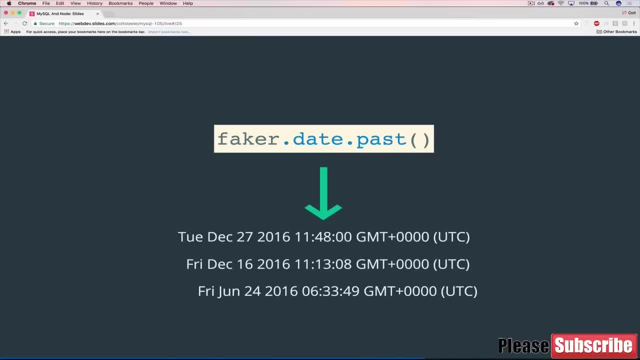 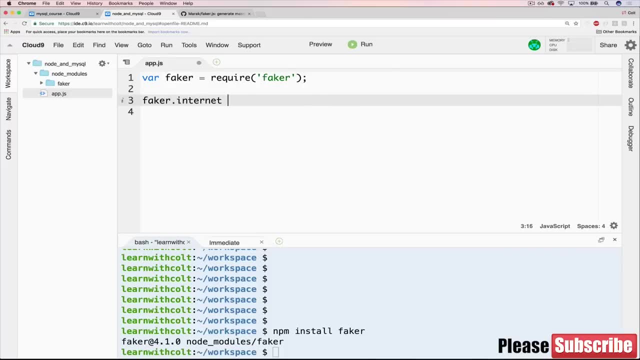 So it will generate things like this. So we also don't want to have to do that ourselves. So let's start with FAKERinternetemail, And we need parentheses at the end, Sort of like MySQL. It's a function We're telling it to execute. 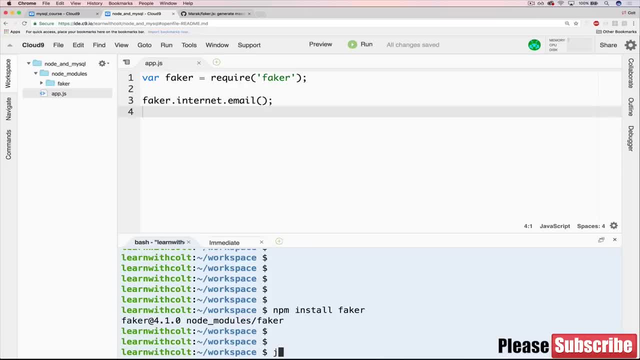 If I just do it on its own And I run the file now, Which is appjs, Nothing happens. Well, that's a lie. It does happen. This runs, But we don't see the result, And that's because we need to print it. 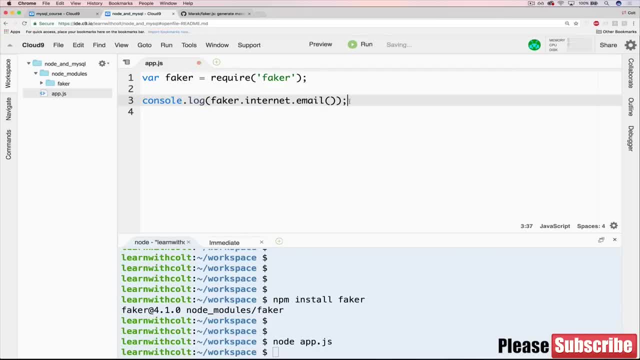 So we can do console dot log Like this. There we go. Now, If I run it again, I see: Okay, We get a new email: Jared Leila, Leila, Trevor, Whatever. So we're getting these fake emails. 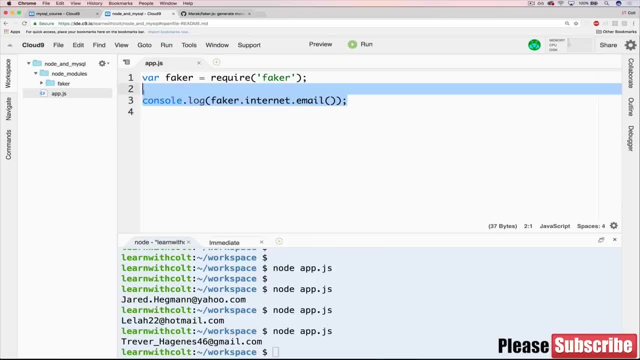 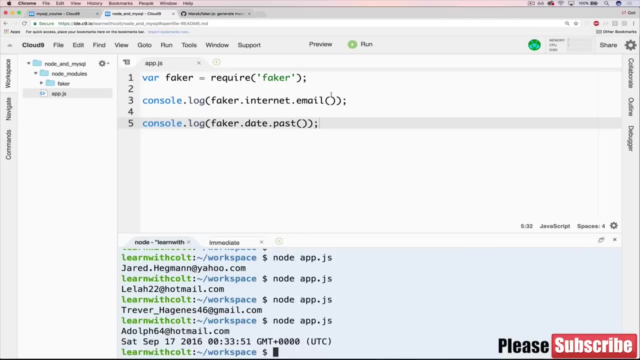 We're going to use that along with. I'm going to copy this and do FAKER, dot date dot past, Which is the other thing I showed you. We're going to use those two to generate 500 users. So basically, this is one user. 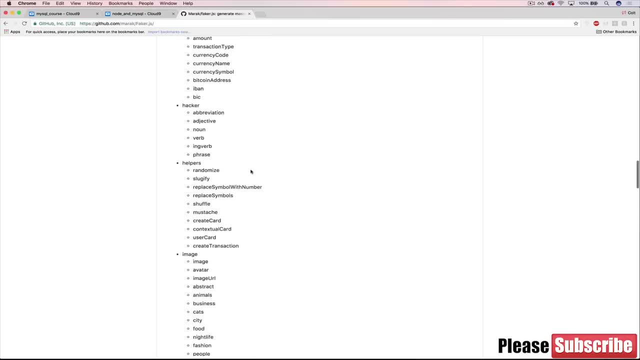 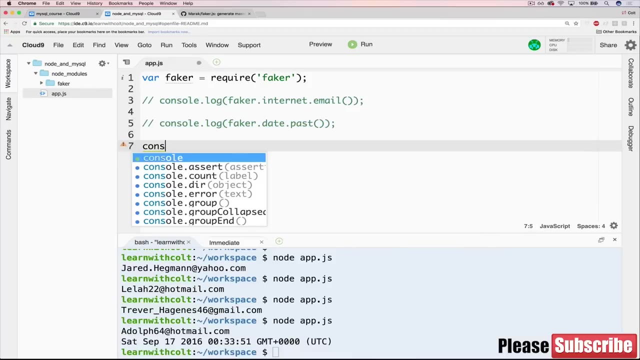 So it's kind of fun to play around with FAKER. You know, dot, hacker, dot abbreviation Or finance, dot currency symbol Or bitcoin address. Let's do address and then city, So we can do Get rid of these two for now. 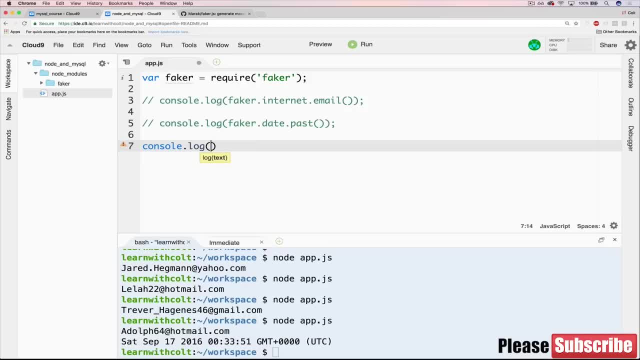 Console dot log, FAKER dot address, dot city. And if we save and run that There we go Robertoville. And if we tried it again We get something different: New Alexandro Fort. So that's the basics of FAKER. 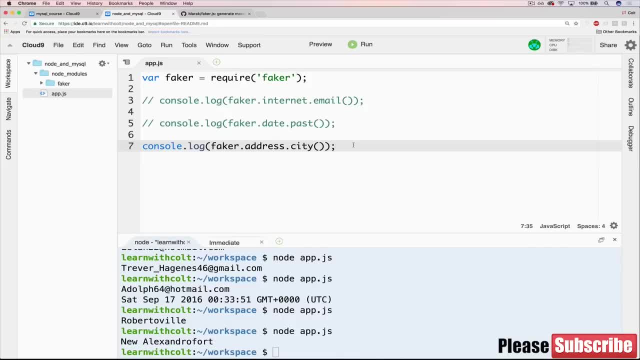 I will show you. So if you already know JavaScript, Skip this section. But I just want to show a bit more Sort of the extended version of Crash Course and Node How we can string things together And make more complex logic. So let's say I wanted to generate a complete address. 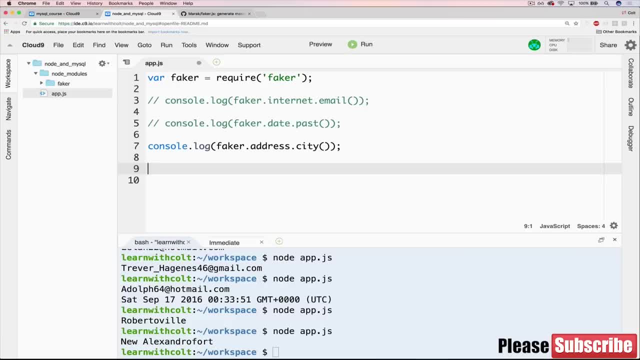 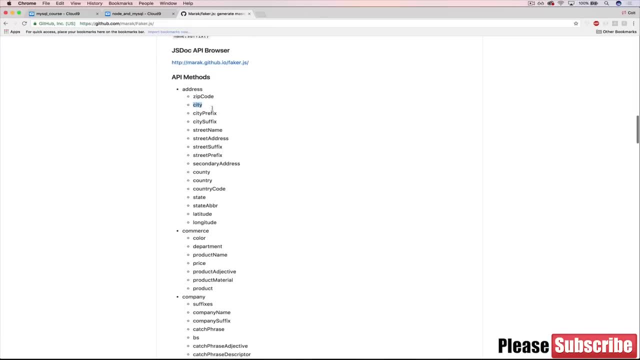 So I wanted You know a number And the street And the city. Let's start with those three. So FAKER has ways of doing that. We've got What do we have? Street name and street address, So let's start with that. 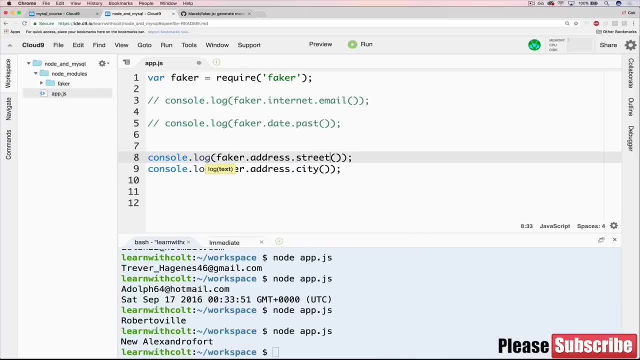 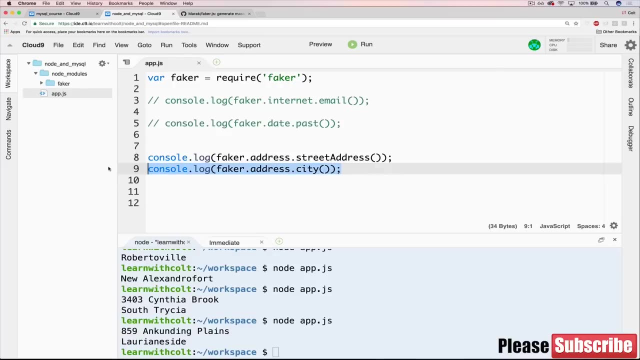 Got FAKER dot address, dot Street Address. Let's start there And run this again. Okay, So there we go. That's working. Then we've got the city Right. And then let's say we wanted to do a state as well. 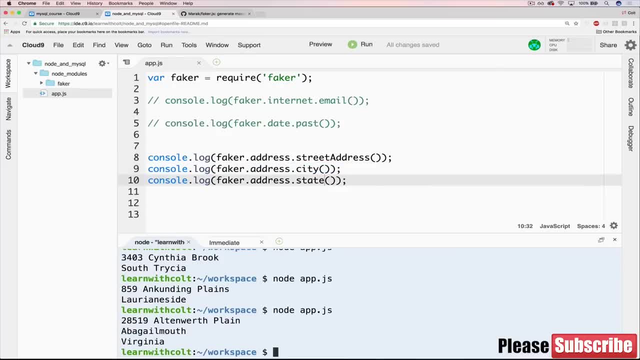 If we're working in the US, Perfect. So here's a complete address Right Now. every time, Let's say, I want three different addresses, I would have to copy these lines like that, Which is not the end of the world. 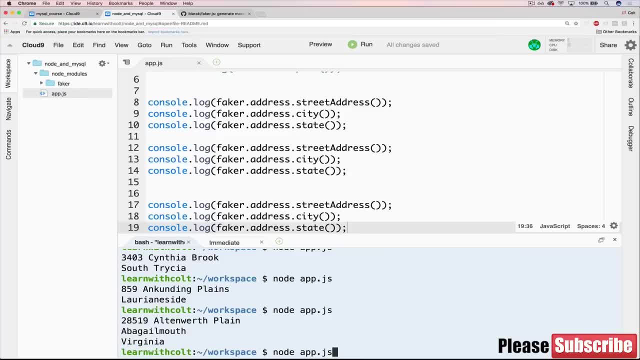 Right, We can copy lines, But there's a much better way of doing this, So what we could do instead Is create what's known as a function, And I'll just call this Generate Address. Think of this as a way of reusing our code. 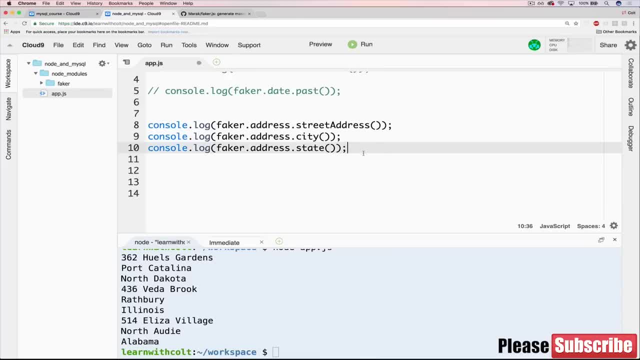 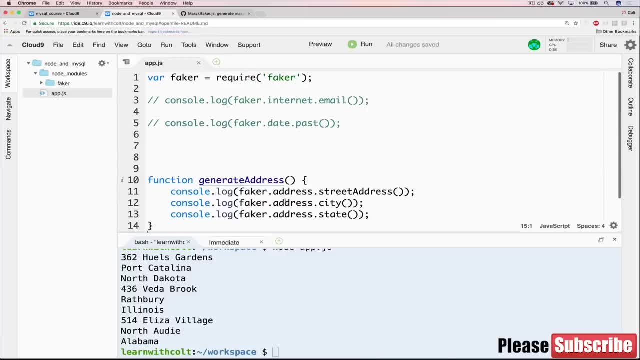 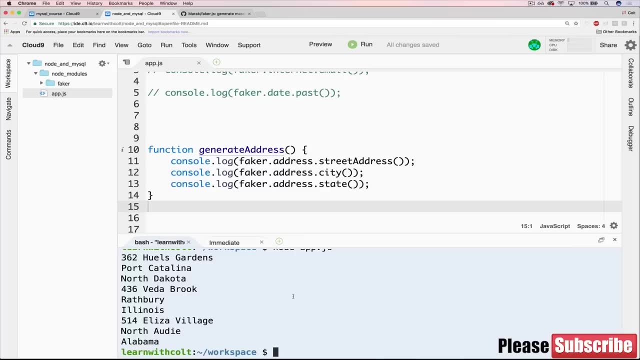 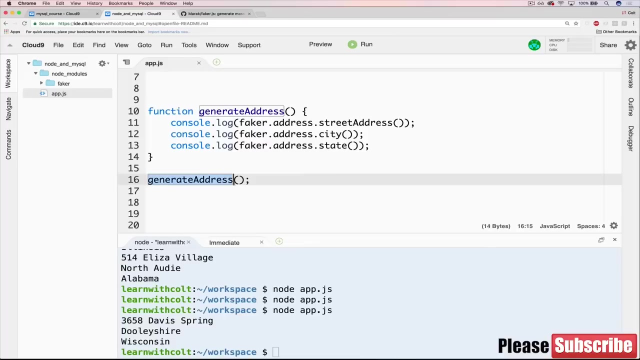 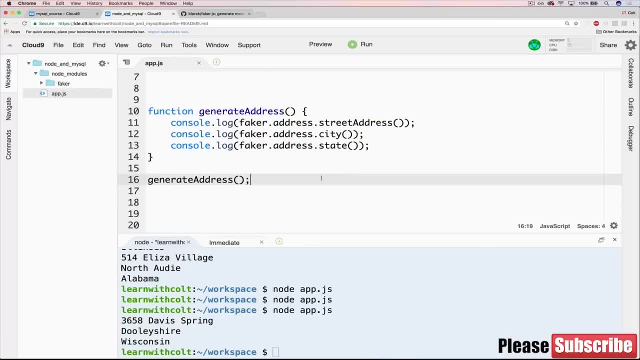 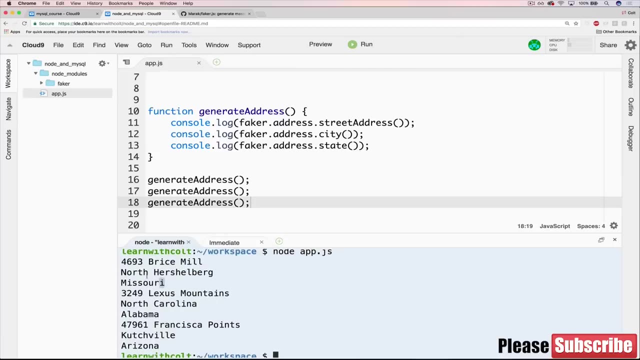 is all right. well, let's run the three lines inside of it. so if I ran this three times, now it's only three lines to do that and we get three different addresses. of course we might want to, you know, compile these together so that they're not on three separate lines. maybe you want commas. 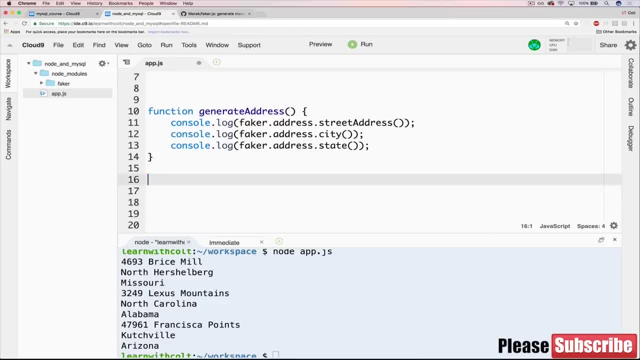 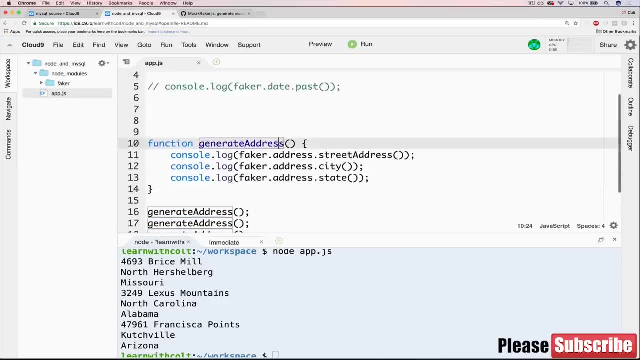 between them. we could really improve it, but the point is that that's basically how you define a function, and we'll be working with functions later on, but for now, that's all I'm going to show. okay, so that's the basics of faker, the basics of packages. we'll be installing other packages. 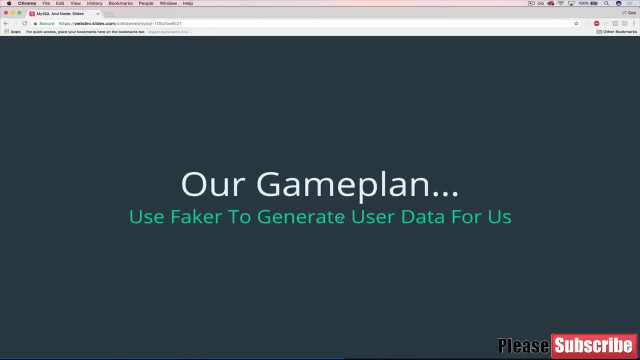 as well as the basics of node. okay, so we saw the very basics of using faker. really just a single line. you know it's a thing and that it's a package. now our game plan from here on out is to use faker to generate our data, for us get 500. 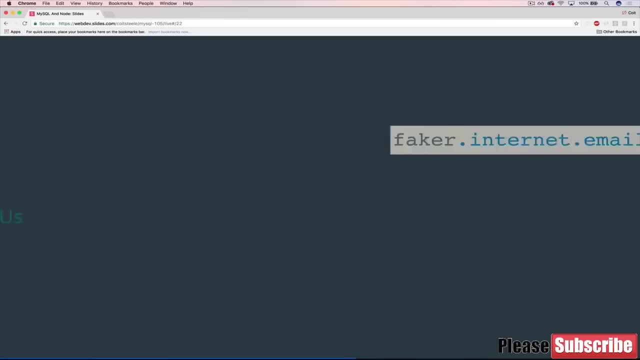 users in there, but faker on its own won't do that, so we'll use this fakerinternetemail. we want one of those, or we want 500 of those actually- and we'll use the datepast. and the reason we need to use datepast is that when a user is created- yes, you know in the real world. 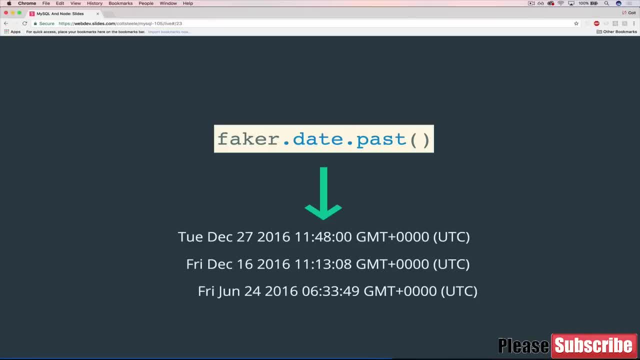 we want to store the current time when they actually signed up. but when we're inserting 500 fake users, we don't want them all to have the exact same time that they're joining, because then that throws off our data right having 500 users who joined at the same exact. 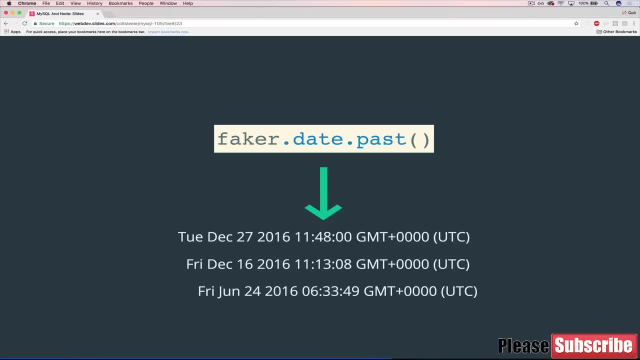 instant, so we'd much rather spread them out so that we could try certain things with the data play around with it. so we're going to generate dates using this. so then the next logical question is: okay, we know how to generate a single email in a single date. how do we do 500 of them? and 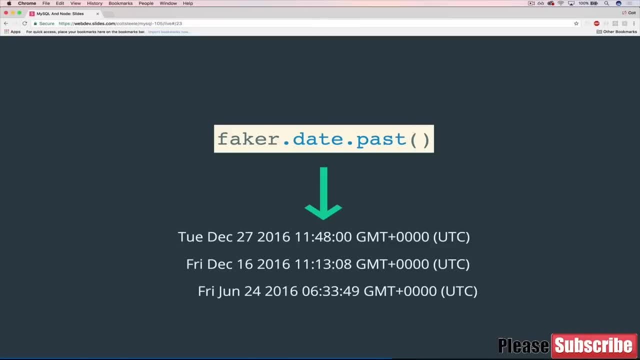 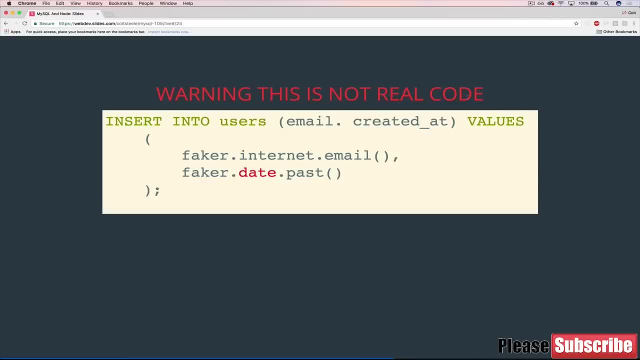 more importantly, how the heck do we get them in a mysql database? so warning up here, red letters. this is not really code that will work. well, it's not code that will work, that will work at all, but i just wanted to show you we would want to do something like this right: insert into users email and create it at and. 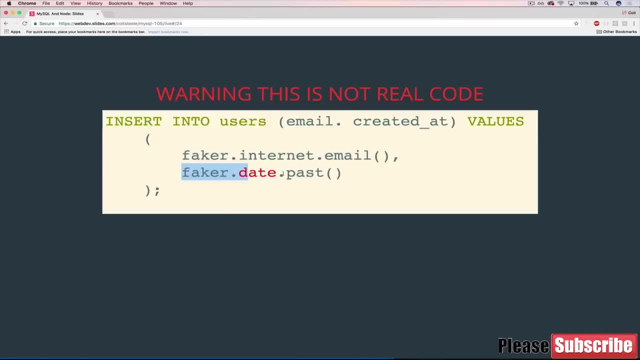 the values. you want a fakerinternetemail and fakerdatepast. this is sort of a hybrid between mysql and node. unfortunately, this doesn't work, but this is what we're going for, right? we want to do something like this: insert 500 of these where we get a fake email and a fake date. 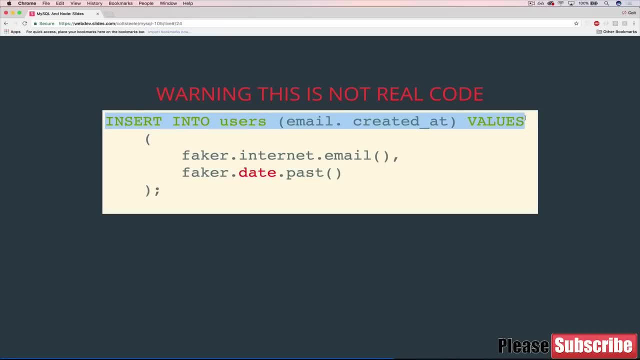 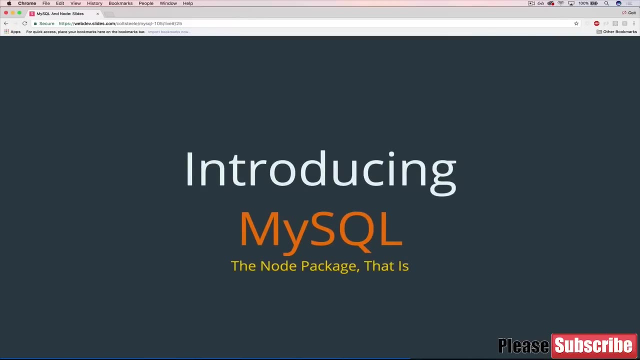 the problem is insert into users. this syntax only exists in mysql and faker only exists in node. so how do we bridge that connection? oh, and we want to do that 500 times. right? the answer is that we use something called mysql, and it's confusing because it's a node package like faker. it's. 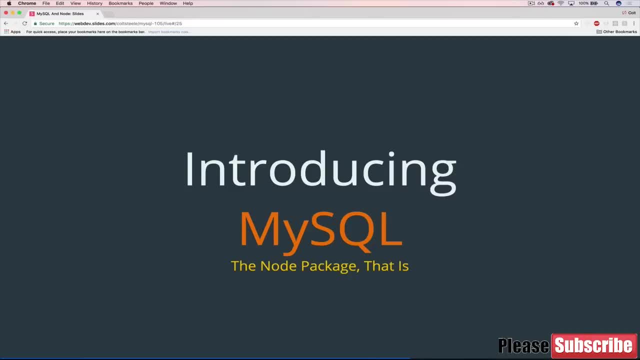 another package called mysql. what it does is it connects to mysql. the actual database talks to it. so every language there are a couple different packages. you know, php has a way of talking to mysql, ruby has a couple ways. they are kind of adapters. think of it as a connector. 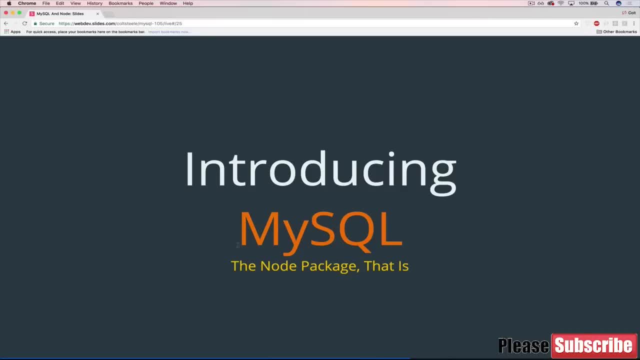 between the two, a tube or a pipeline, and there's a couple for node, but the one we're using is the most popular. it's called mysql, which personally i find kind of confusing. i wish it was called, you know, mysql node, or mysql connector, or mysql js or something. 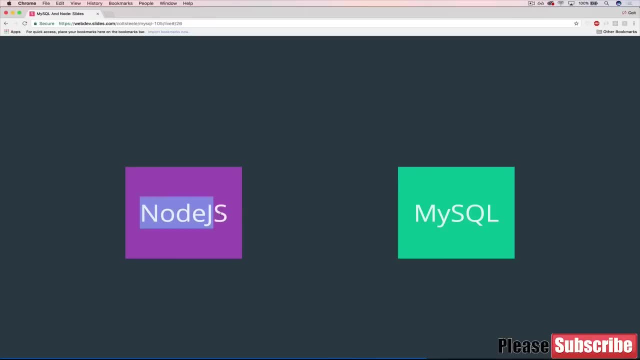 here's a couple diagrams of basically how it works. so we have node on its own- this is where we've been working- and then we have mysql on its own, our separate database. so this has our data stored in it and the mysql package will be able to say things like: hey, mysql database, how many? 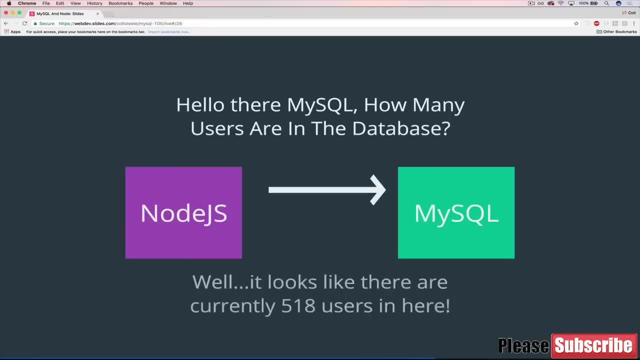 users are in there, ask it to the database and then the mysql database will be able to say: well, looks like there are currently 518 users, send that back to node and we can use it, or it might be something like this: hey there, mysql database, how many users are in? 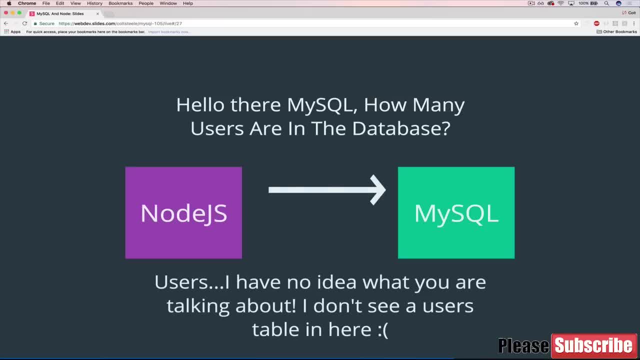 there and mysql might say users. i have no idea what you're talking about. i don't have a users table in here, in which case we would get that back to nodejs and we'd be able to know that because of the package we're using. mysql package is both asking the questions, right, it's querying. 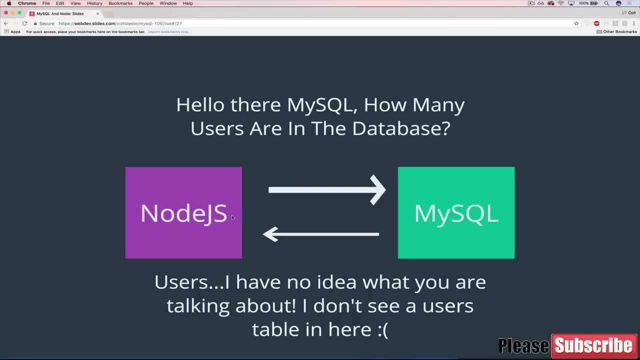 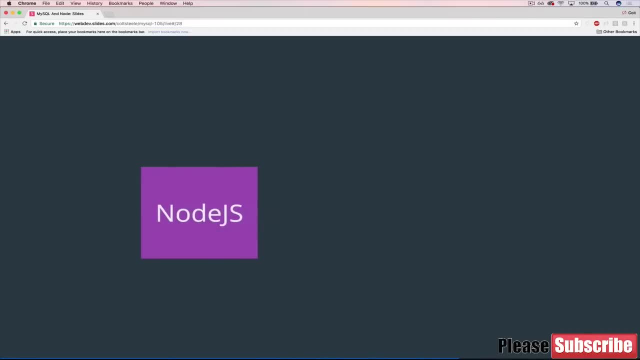 the answer. so then in here we can write logic that says: okay, if we don't get a response, if there's an error message, let's do one thing, otherwise do something else. or a third scenario: hey there, mysql, our adapter, our mysql connector, might ask how many users are in your database. 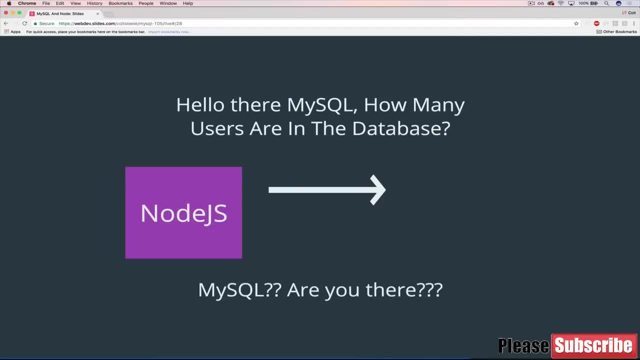 and there's no database, we don't get a response. well, we need to figure out how to handle that node and fortunately, fortunately, the mysql package handles that and we can do that in nodejs. so it will, you know. start by freaking out. are you there? what's going on? a bunch of sad faces. 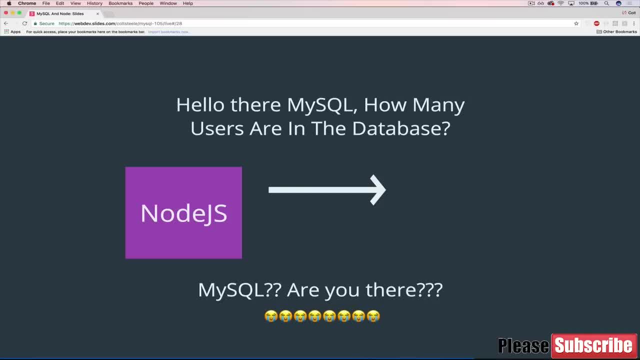 but then it will figure it out. it will basically time out and it will figure out: there's no connection, there's no database there, and we'll be able to handle that as well, which is something that could happen. your database server could go down, something could go wrong. so these are. 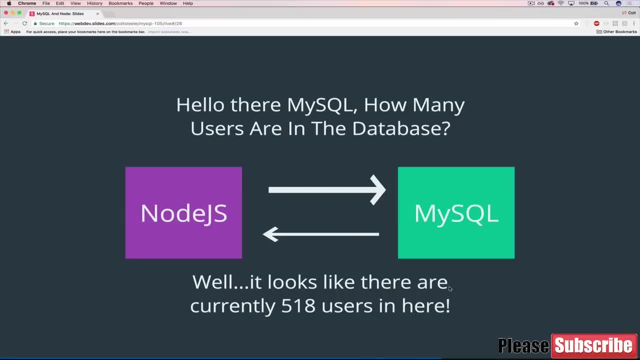 different scenarios. mainly, we're working with this one right, where there's good communication and everything's working how it should, but the key thing is that we're not going to be able to work with the end users anymore. the key thing is that the package- mysql package- works in node. 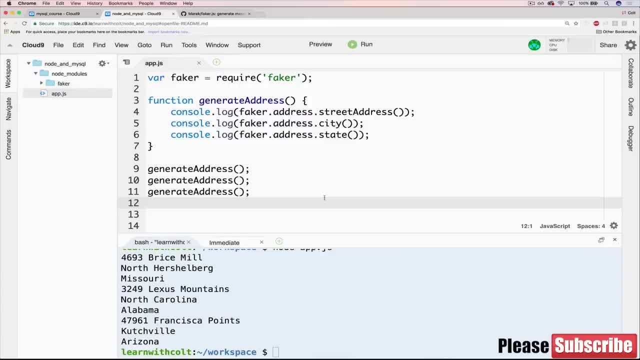 talks to a database. so, without further ado, let's see how that works. all right, so we're back here now and our goal for this video- i'll just lay it out there- is to have communication established between a mysql database and this file of javascript of node. it's not going to be crazy. 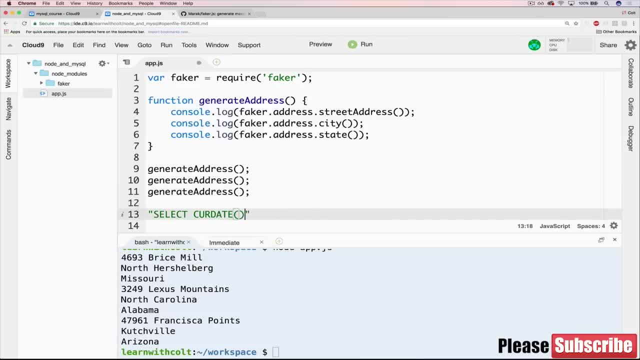 we're just going to be basically running a very simple query like this: select. we could do curr date, Or we could do something even sillier like select 1 plus 4.. But those are SQL queries that we could run in a MySQL database and get an answer. 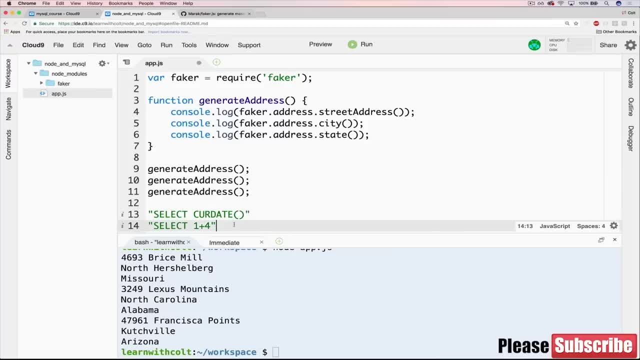 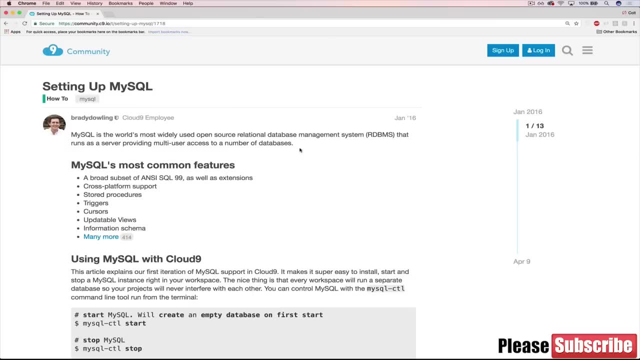 So we're going to run them from this file, And to do that we need to first establish a connection, And even before that, we have a bigger thing to take care of, which is that we don't have MySQL set up in this Cloud9 instance. 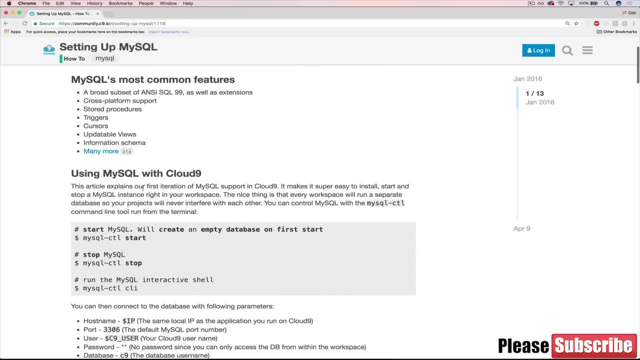 So if I'm back in the Cloud9 docs, you can see remember when we ran this very, very early on mysql-ctl start And what it does is it starts MySQL in the current workspace that you're in. And if you read this note, it says: the nice thing is that every workspace will run a separate database. 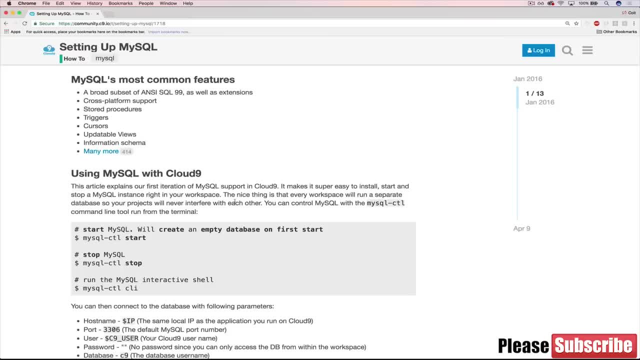 so your projects will never interfere with each other, And that's really nice and useful. But what that means is none of our data from our previous workspace is available here, So all we need to do is just run this command. So we'll do that now. 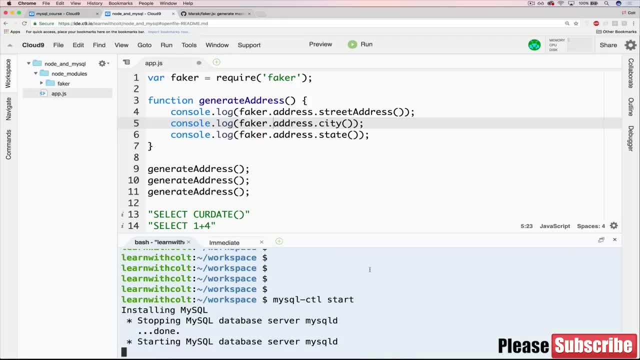 Here I am in Cloud9.. I'm just going to run it And all that we should see is that it installs MySQL. Everything's good, But something to take note of right now: the root user. So we need to remember this. 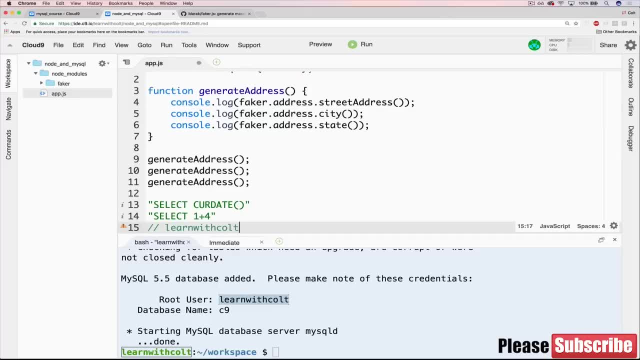 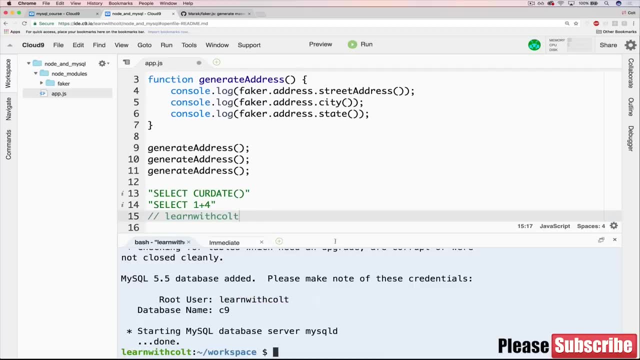 And you'll see why in just a moment. So I'll just put a note down there. Don't make fun of my username, please. I regret it deeply, But it's here to stay. Learn with Colt. Yours will be something different, but we need that credential. 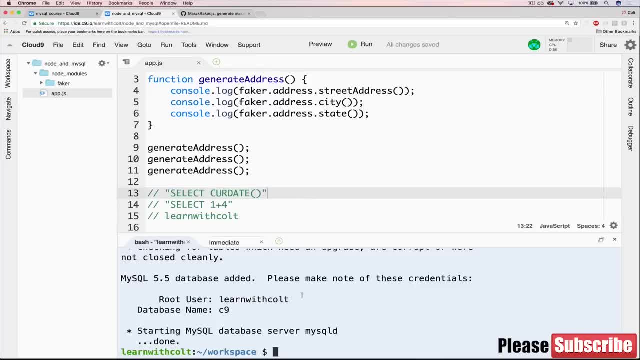 Okay. So then the next thing: we now have a MySQL database. I'm going to open up a new terminal over here and just keep it open, And we're going to connect to the CLI. Remember how we do that. It's mysql-ctl space- CLI. 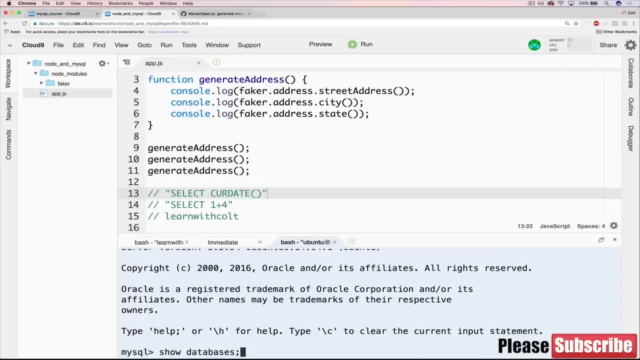 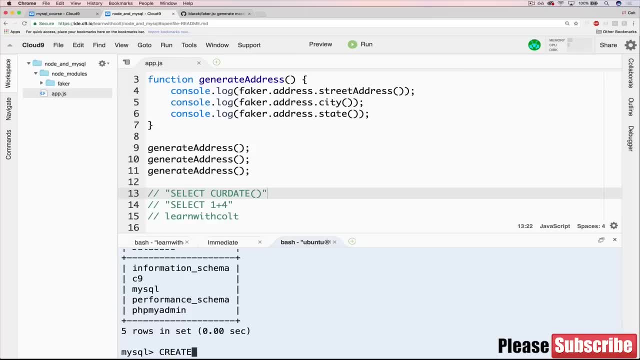 Okay, And if we look at databases, we have nothing really. We have these kind of basic ones that we get from Cloud9.. Let's create a new database And we'll just call it. join Us, Already forgetting the semicolons. 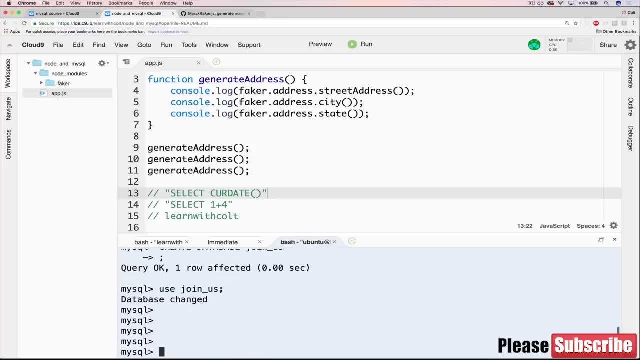 Okay, And then we'll use join us, just like that. So we have a database And just to show you, you know, if we run a command like this- select cur date, we get an answer. Or if we do select one plus four and add a semicolon, we get an answer. 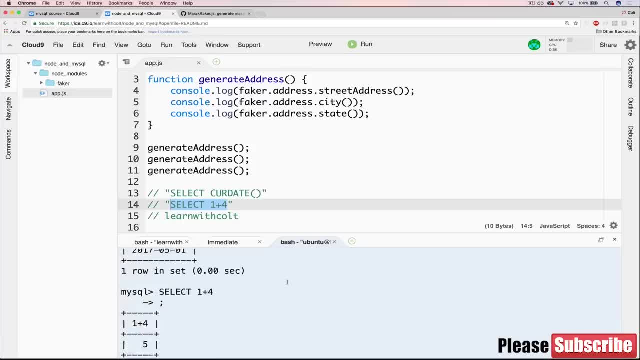 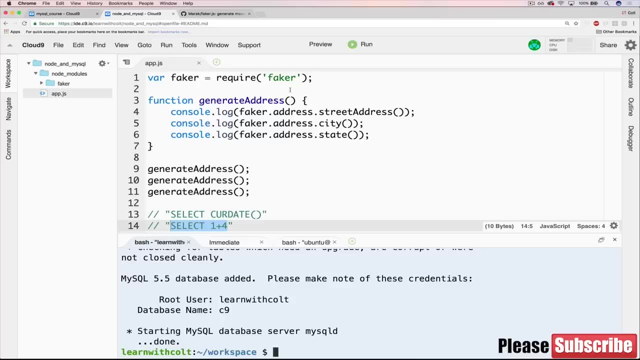 So this is in MySQL. Hopefully that's no surprise that that works. Now the question is: how do we get this file, which is not SQL at all, It's JavaScript. How do I get it to talk to the MySQL server that's running and run some code in it? 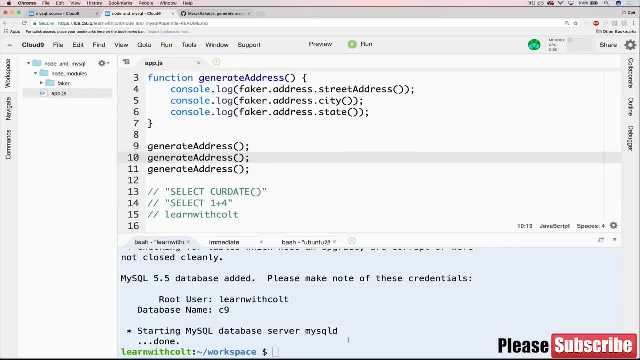 And there's a couple of components to that answer. The first thing we have to do is install the package. So, just like before, it's npm install, But instead of faker, we type mysql. It's the name of the package. We hit enter. 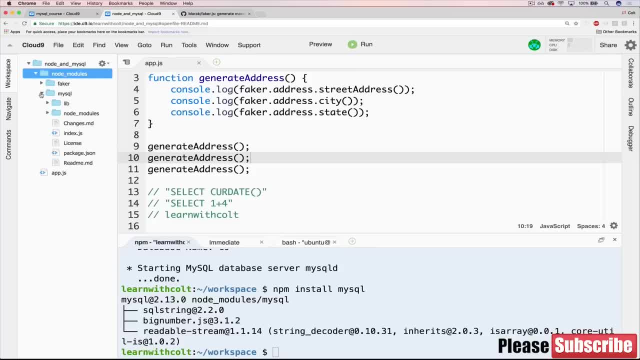 And once it finishes, if you open up node modules, there's a new MySQL folder. So this is the code that connects. So on it On its own. it's not doing any connecting right now. It's a library, It's a tool set that we can utilize. 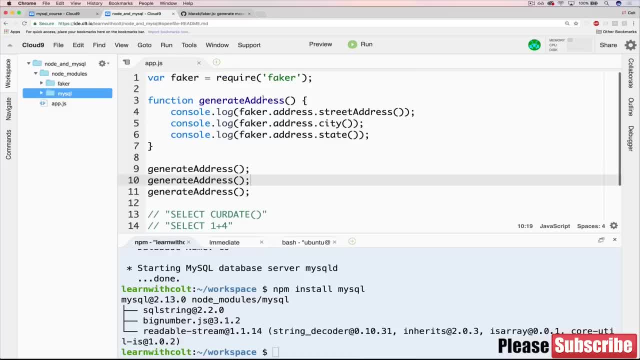 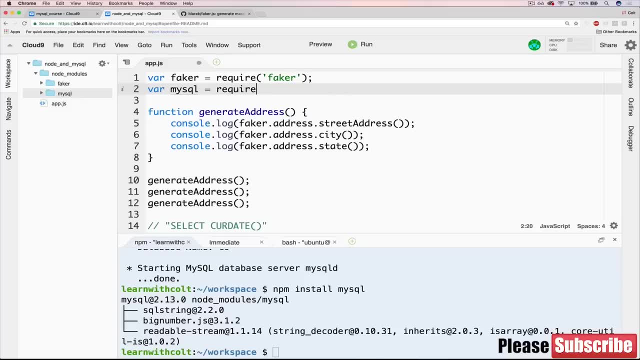 But we have it on our machine Now we have it in Cloud9. So I'm going to come up here and require it, just like I did for faker. I'll type mysql equals, require mysql. if I can type, That on its own doesn't do anything. 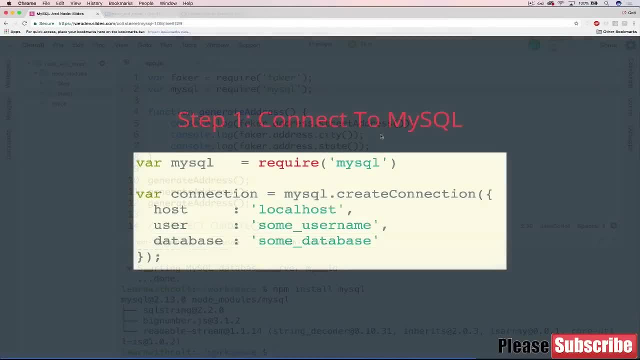 Well, that's a lie, but it doesn't actually talk to our database in any way. There's a bit more We need to do, And it looks like this. So what we do is establish a connection with the database, So we require this first. 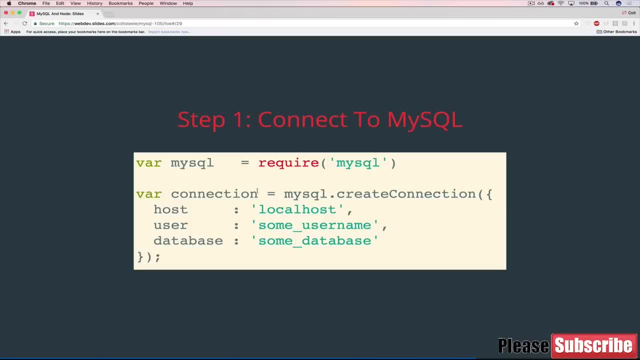 We require mysql. We save it to a variable, Then we run mysqlcreateConnection, which is a method that it comes with, And we have to tell it a host, which we'll go over later. We're leaving it as local host. 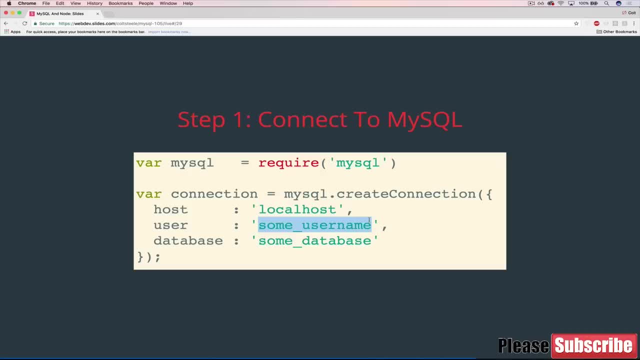 Then user, which is going to be whatever your username was- Mine was learnwithcolt- And then a database name. So we just made a new database. I think it was called join us. That's the one we want to work with. 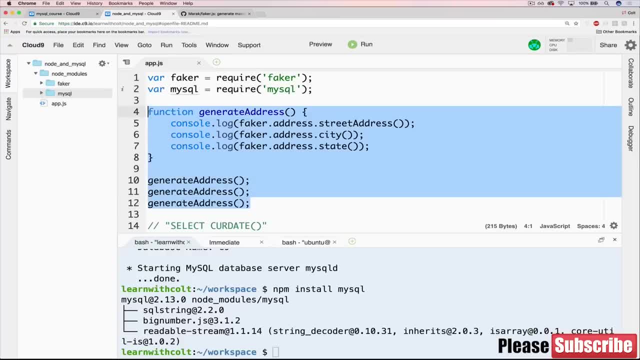 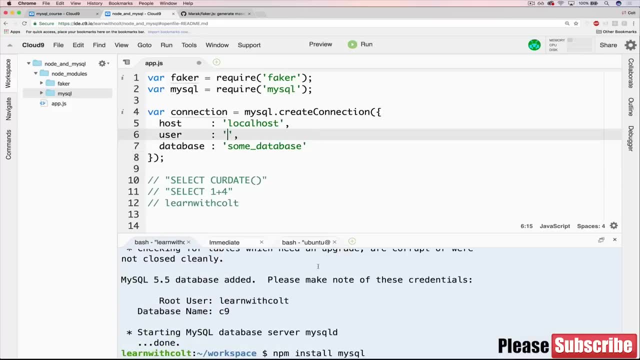 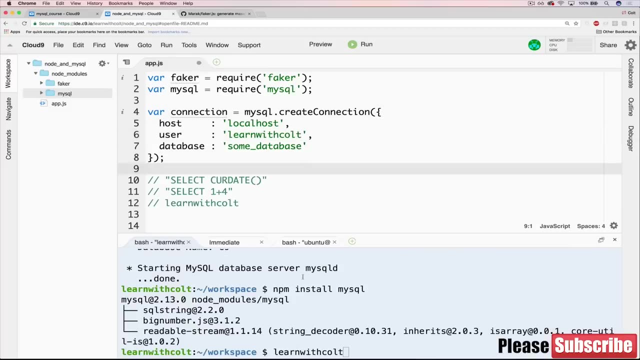 So if we copy this over, I'm going to get rid of our generate address. for now, I need to fill this in. So some username for me is this right here: learnwithcolt. That is what mysql is expecting. It says: please make note of these credentials. 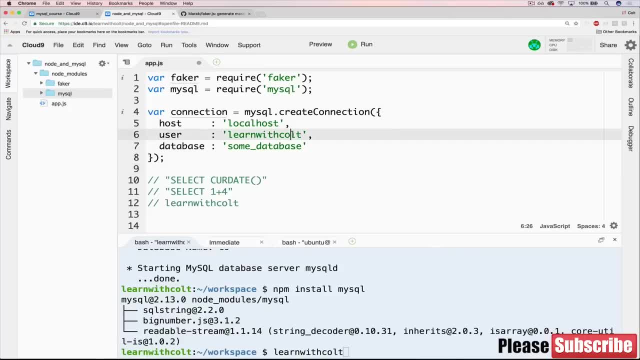 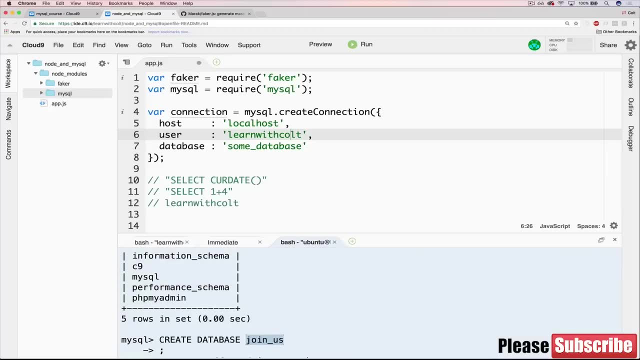 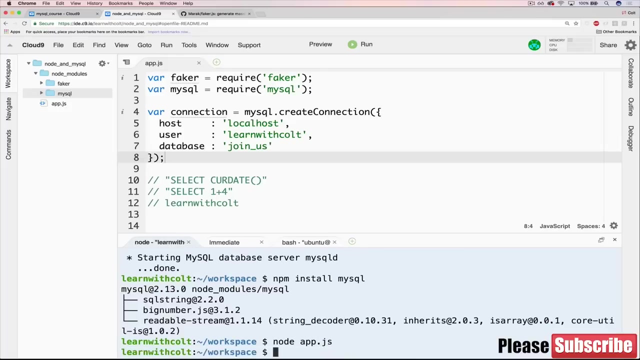 We want to keep track of that, Okay, So we put that in there, And then the database that we want to use is the one we just created, which was called join underscore us, Just like that. So if we try this right now, we try running this file, node appjs- nothing happens. 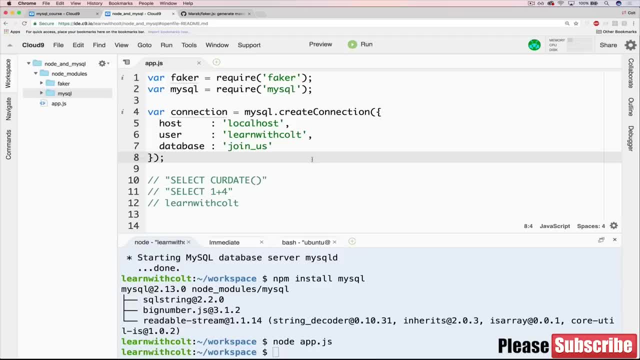 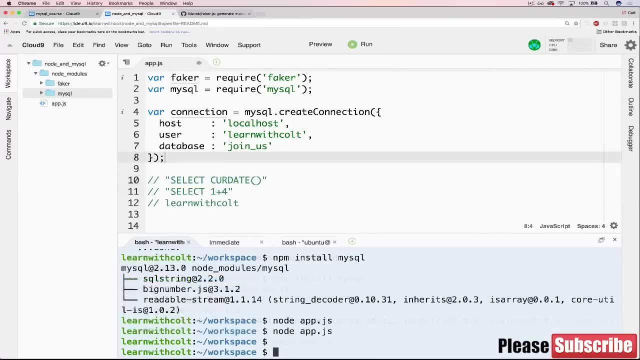 And that's actually a good sign. That means that there wasn't a problem, But at the same time, we're not running any SQL code. The point was: by the end of this video, we want to do something like this. So then the next thing to do that looks like this: 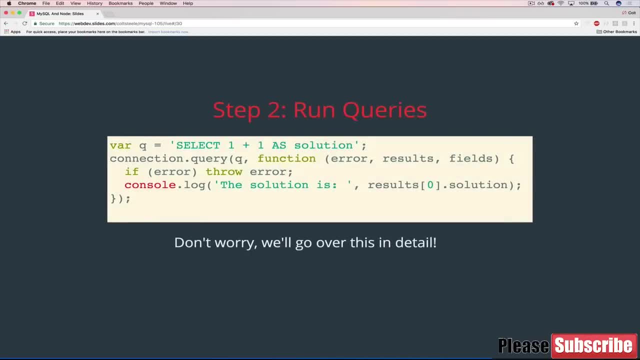 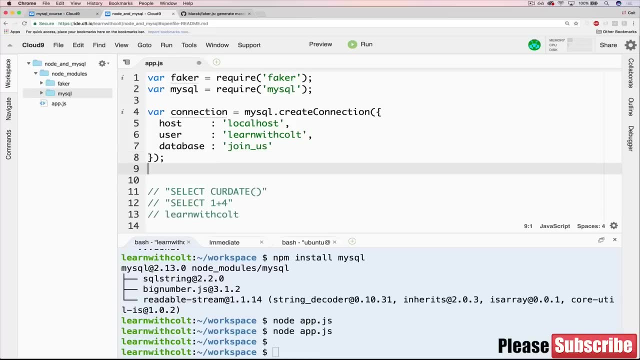 And there's a lot to take in here. Totally understand that We're going to start by just copying this over or you can type it as well, But this is how we run queries. Okay, So there's a lot. First thing I'll show you is: we have a query. 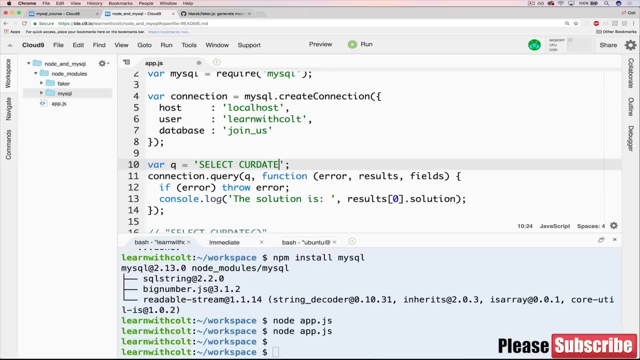 I'll just do select. Let's do curdate. That's more Accessible. So we write our SQL code in here. Okay, so we could do whatever SQL we want. We don't have any tables yet in there, so we're not going to work with tables, but we could do something like this, like curdate. 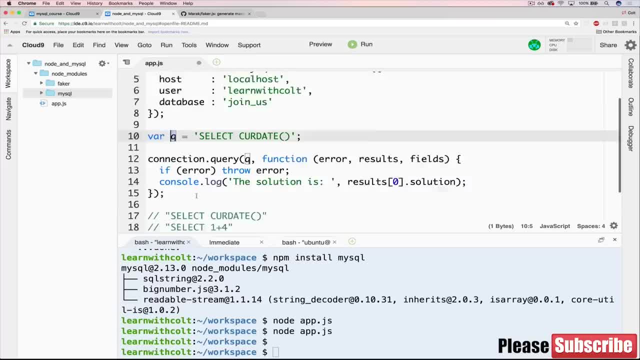 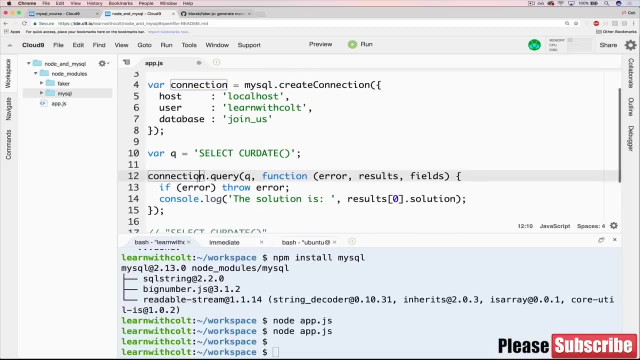 Then we just save that to a variable called queue. Now this is the trickier part. So we've got connection that this is our connection we created. So we're referencing it. connection dot query. We're telling it to run the query queue. 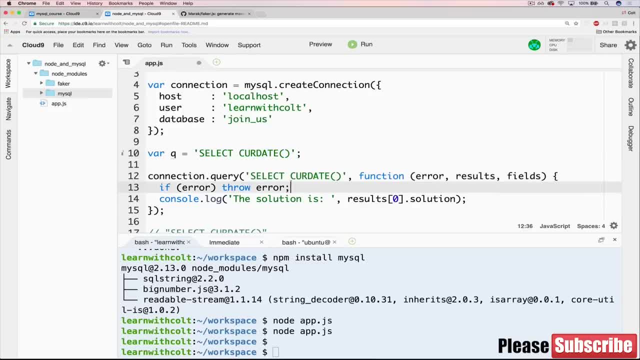 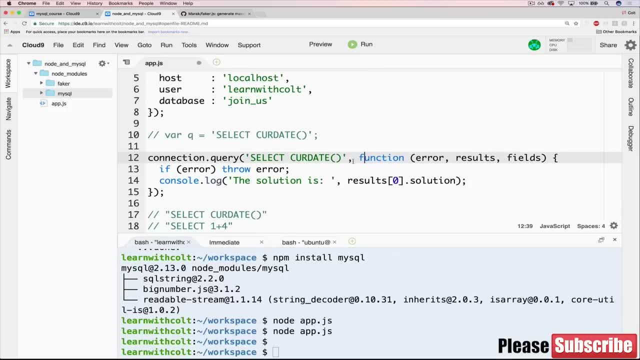 So I could have just taken this And put it directly here. Just makes it a little longer of a line to look at. But I'll do that to consolidate it and to show you that it works. Then we have this whole function- error results, fields- kind of a mess here. 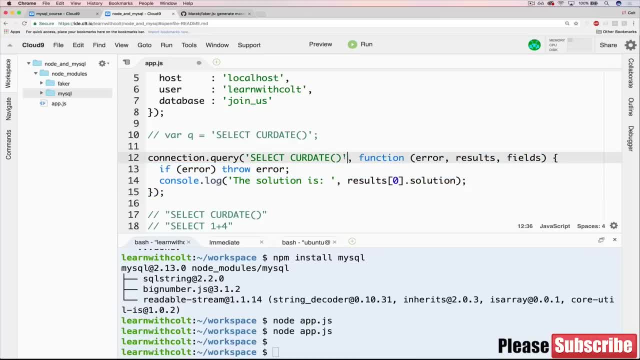 It's a lot to look at. What this is saying is when this query is finished. So we're going to reach out to our database over here. We're going to try running select curdate And if we just run it here you can see it works. 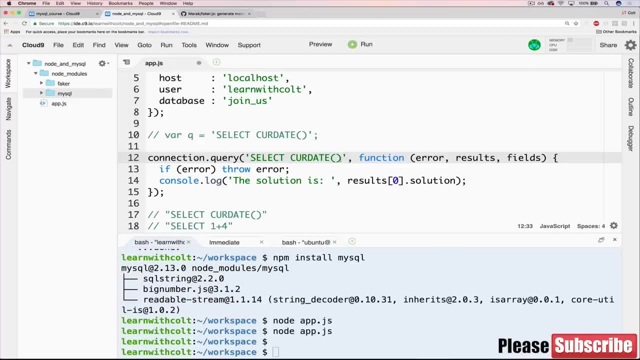 So if we try running it from this connection, Whatever happens when it's done, run all of this code. here It's called a callback And again I wish I could go into more detail. but basically this will run And if there is an error there will be something stored in error here. 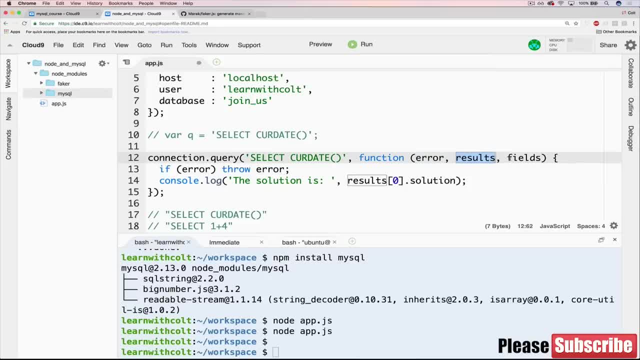 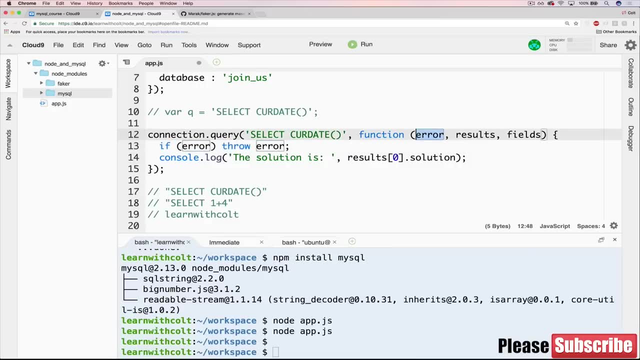 If we get results, it will be stored in results. We'll talk about fields later. We're not going to use that now. So I have this if statement that just says: if something happened, if there's an error, then just stop, Throw error. 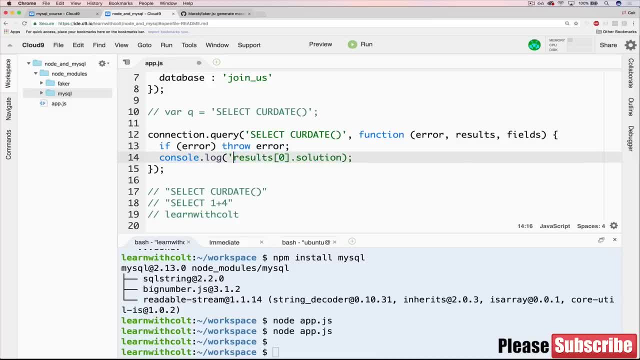 Right there, Otherwise, And we can even get rid of all of this and just print out even more- Let's just get rid of everything and just print results so you can see what we get back, just like that. So there's still a lot going on, I realize. 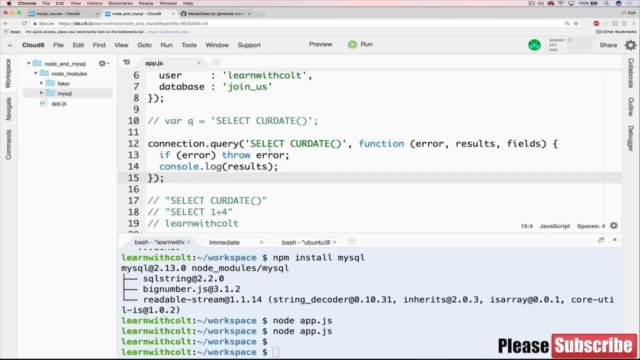 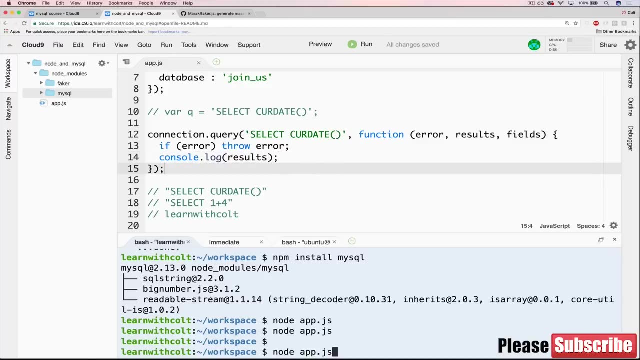 Unfortunately it doesn't get simpler, but hopefully you can see the core idea. We have our query and everything else here is just kind of the JavaScript wrapper around it to run this query, Connect to a database, Run the query. So let's see what happens. 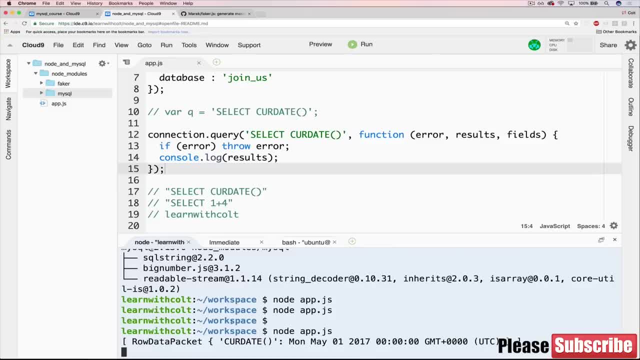 OK. so two things to notice. One: we get this row data packet thing back, We have curDate colon and then the answer for what curDate was, which is great. But then we also have this other thing I don't know if you picked up on. 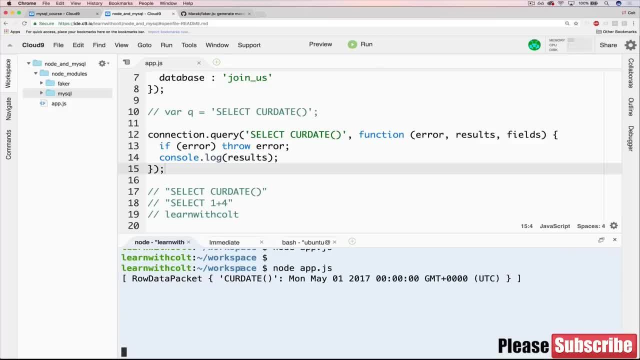 My cursor has changed. I am not in the regular terminal. I have to hit control C to get out of there, And that's because a connection was opened But it actually was never closed and never ended. So it's not a problem, but basically that connection is persisting. 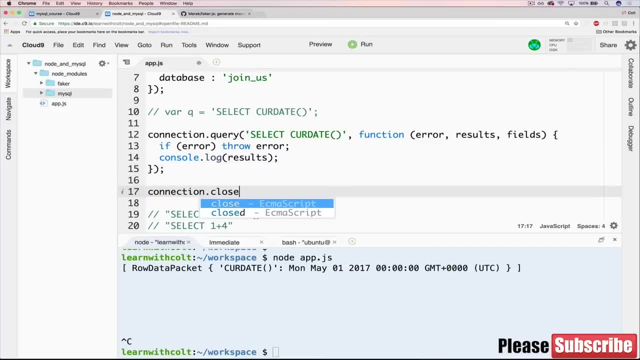 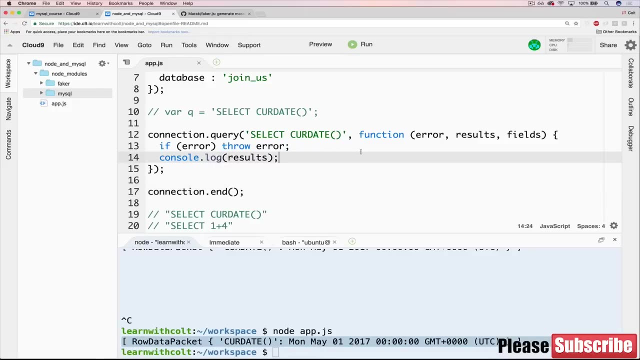 So at the end we can do a connection dot, either close or end. Let's try it again. There we go And it ends now and you can see we're done OK. so now let's talk about our results. First of all, we should pat ourselves on the back for getting this far. 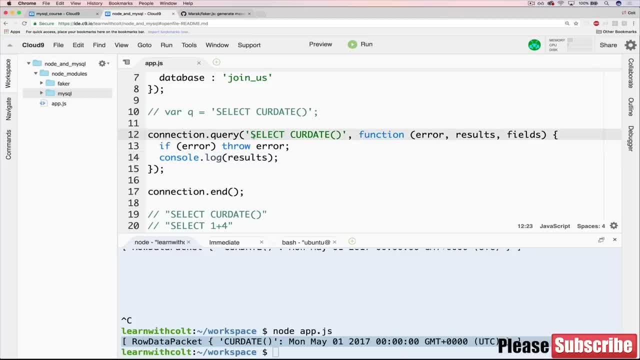 We now are running simple queries, yes, but we're running queries here In this node file. this sets the groundwork for everything else we need to do. So imagine that instead of a single select curDate, what if this was? insert 500 users and we're passing that in. 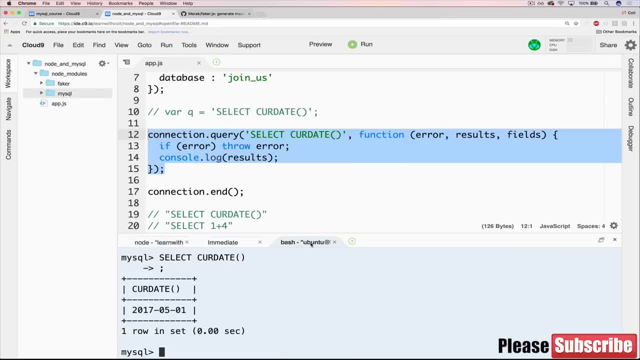 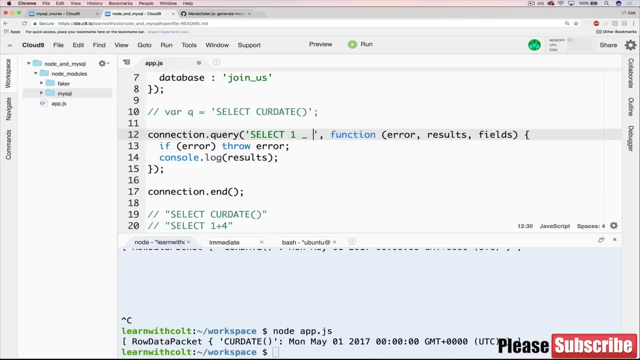 and we're running it from node, talking to our database, which hopefully you think is cool. Let's try changing this to something like select one plus five, Saving it And you can see. we're now getting row data and one plus five colon is six. 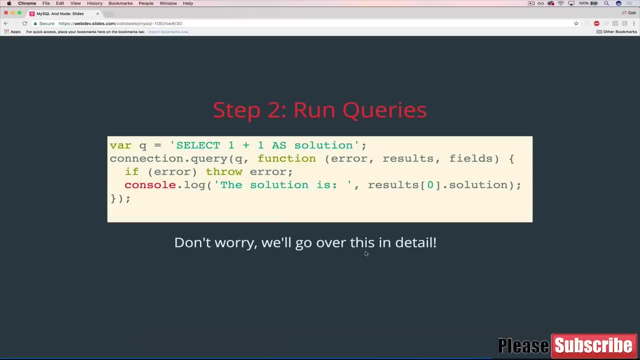 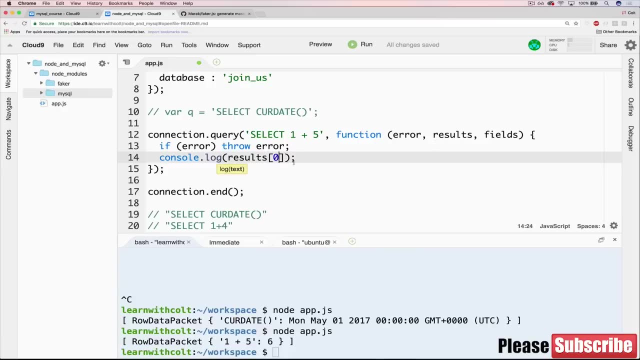 So this what we're getting back. this syntax is kind of wonky. I totally get that. the way we can get around it. If we just want the answer, we can start by adding in zero, which is basically, if you're familiar with an array, it's going to give us the first item. 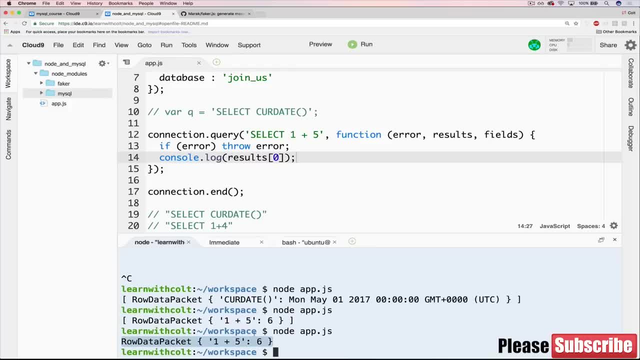 So if we try this again- now we're working with this row data packet in particular and to make this easier to access, I can just go in here and add an as. So if I do as answer, for example, select one plus five as answer. 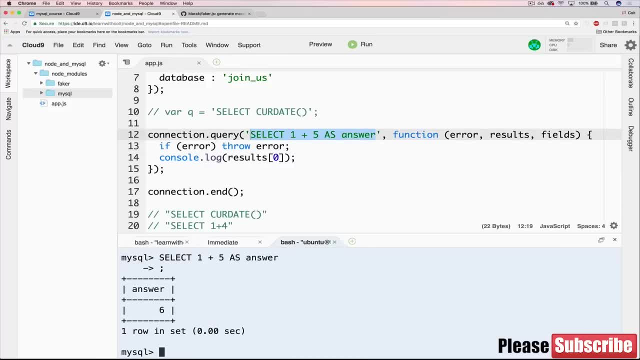 I mean, if we run it over here, This is what we get right. Well, this is not JavaScript. so the whole job of this MySQL library is to, or the package is to, figure out how to take this and turn it into something we can use. 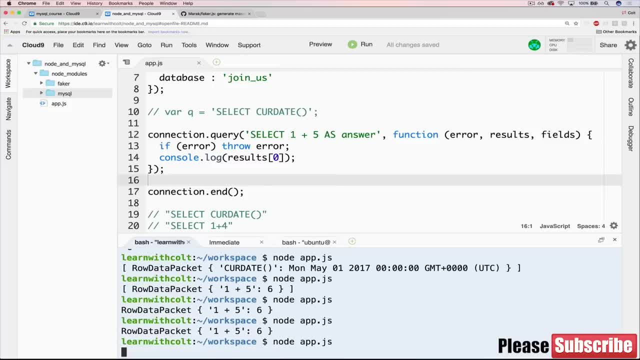 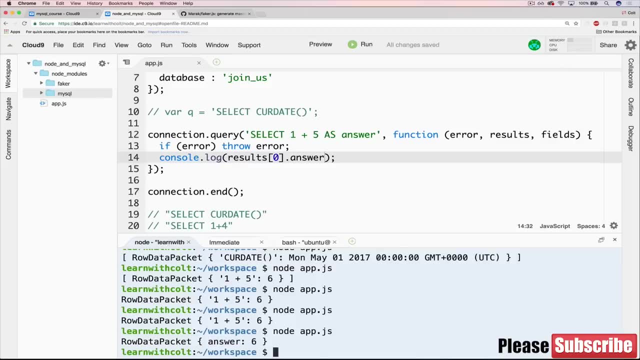 So if I do as answer now, I try it again. You'll see that it's stored now under the keyword answer so I can access it just like that. Perfect. So last thing that I'll show you, let's do select, and I'm going to do this one. 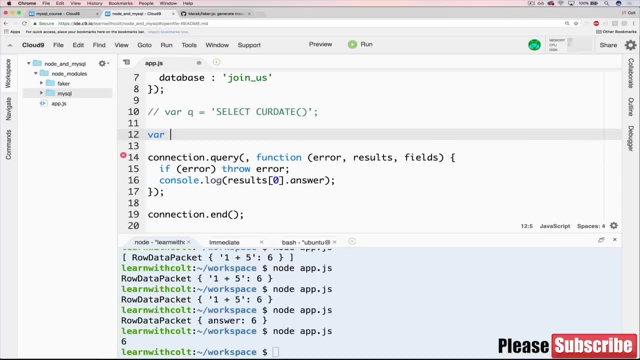 in a separate line or as a separate variable. I'll call it our queue, And instead of just selecting one plus six or one plus five, let's do select cur time as time comma, cur date as date, Then finally Now As now, and I do need that right there too. 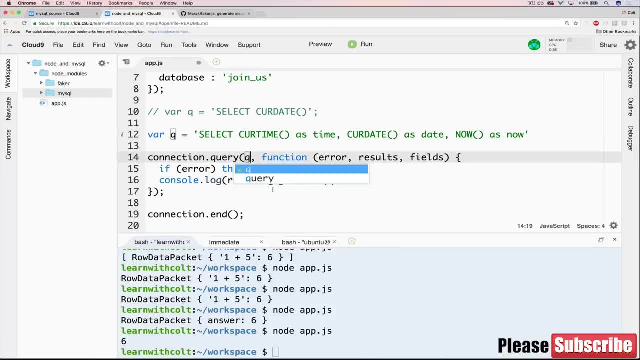 OK. so if we do that- And I put queue here- I'm basically just saving myself from having to make a gigantic line. So by referencing queue is referencing this query, which is very useful. It's going to run it And rather than doing all this, let's just look at results like that. 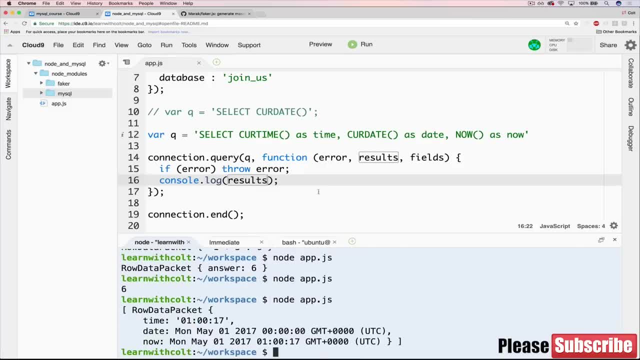 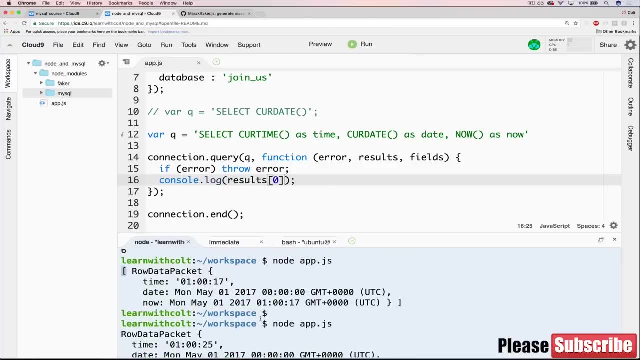 See what we get. OK, now, if you look at our results, we can do results zero, which will just get us basically the same thing, but we don't have this array around it anymore. More importantly, we now have three items coming back which should make sense. 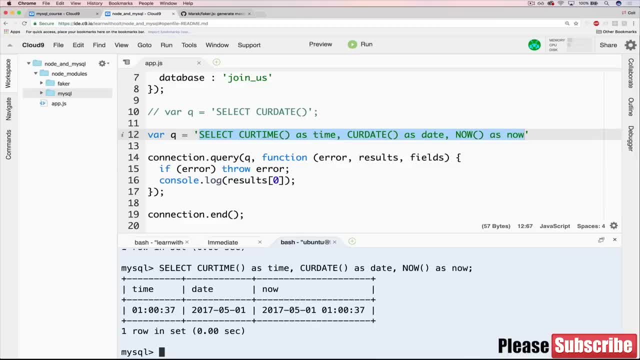 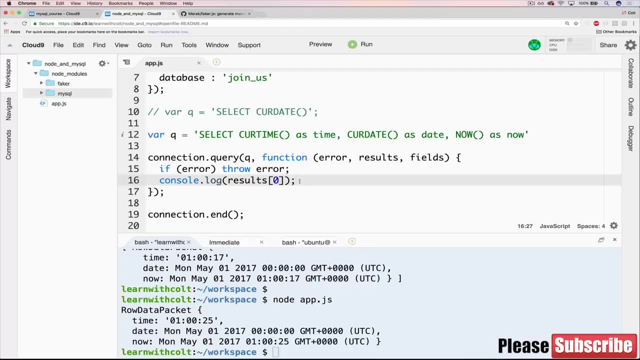 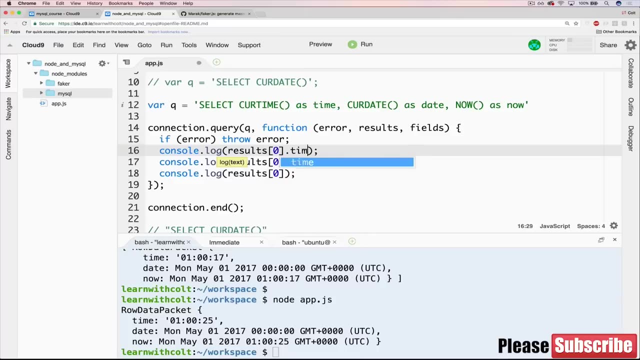 Right, If we went and took this over to my SQL, don't forget the semicolon. This time we get three results: time, date and now. So then the question is: OK, let's print them out all separately. So we'll have three prints, but we need to access them individually. 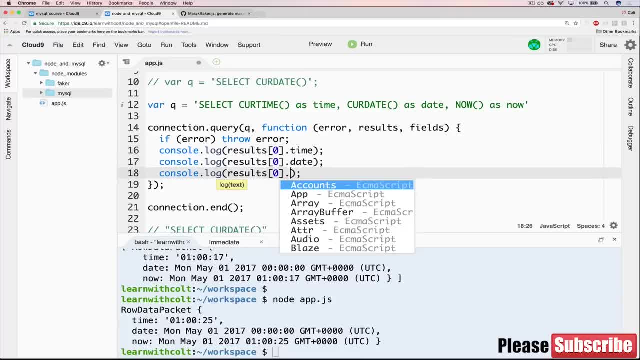 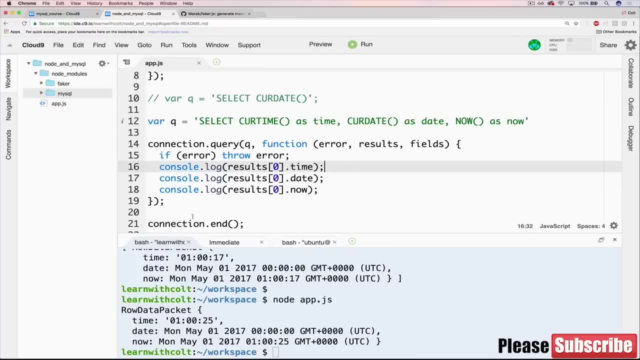 So we'll do time first and then date dot now. So by putting in this alias the as when it comes back from my SQL. So imagine that diagram, we're sending it over, We're saying, hey, please send me, let's say cur time as time. 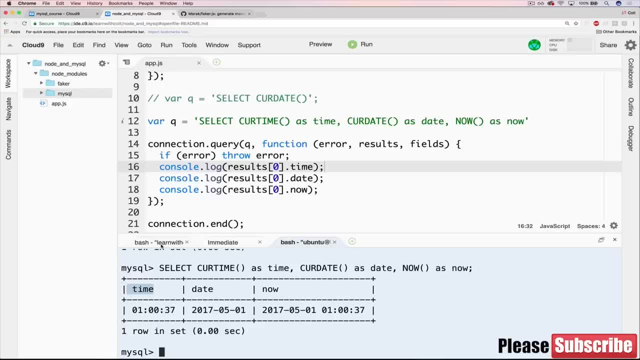 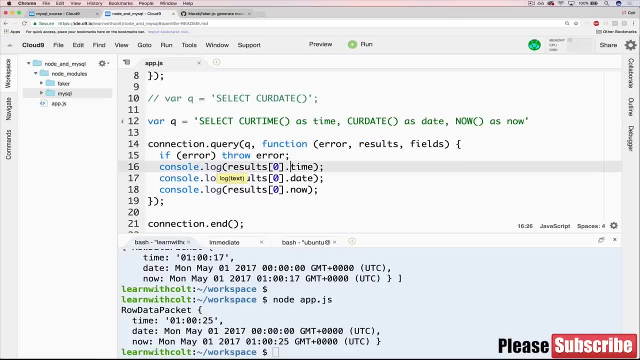 And it does that. OK, here's cur time as time I'm sending it back to you. JavaScript: This JavaScript library takes it takes it in the results under the name time only because we gave it that alias. So whatever I change this to, I would need to access it under that name. 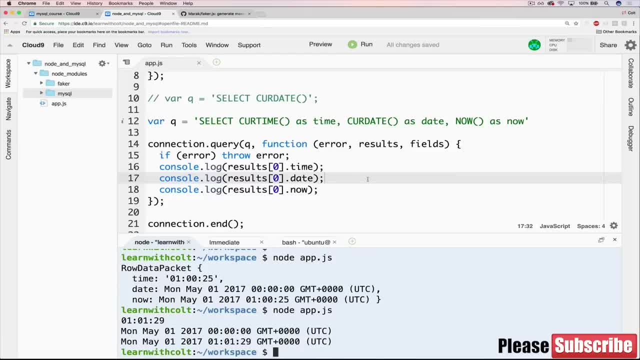 Anyways, now, if we do it, there we go. I'm getting the three different things that we asked for. OK, so that's the extent that we're going to work with it here. Next up, we're going to create our table. 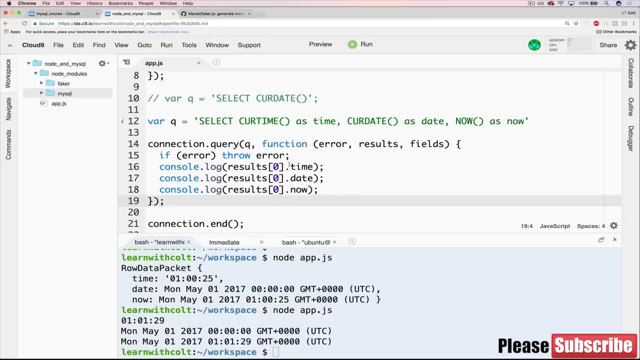 and we're going to see how we start inserting and selecting data from this file. So, rather than just selecting cur time, we're going to actually do something with the database, something that we couldn't do without my SQL. OK, so in the last video we got our node. 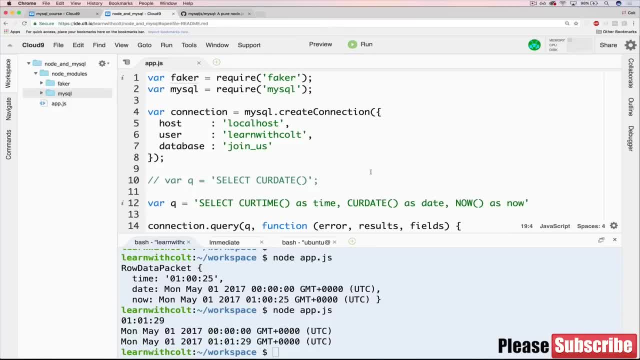 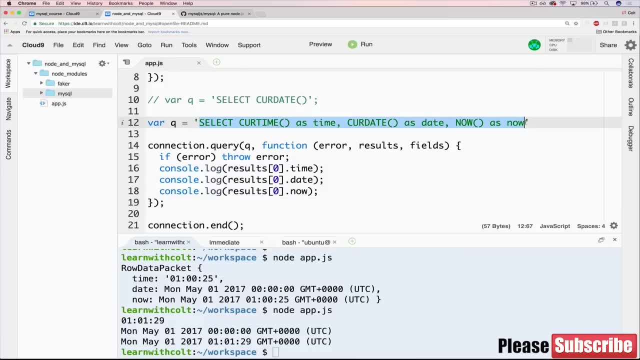 file, JavaScript, communicating with our MySQL database. I'll be a very, very simple communication. We're not actually interacting with tables, but this is SQL code that we're running, So the next step, of course, is getting it to interact with tables. 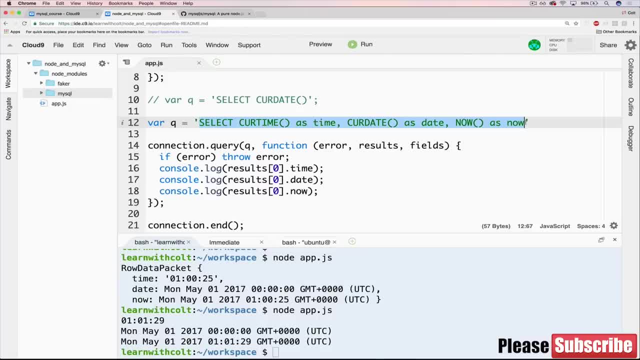 So we're going to in this video, we're going to create our table, We're going to define our schema, create our table in my SQL, separate from JavaScript, And then we're going to try and query it from here. So, basically, we're going to go into my SQL, create our table. 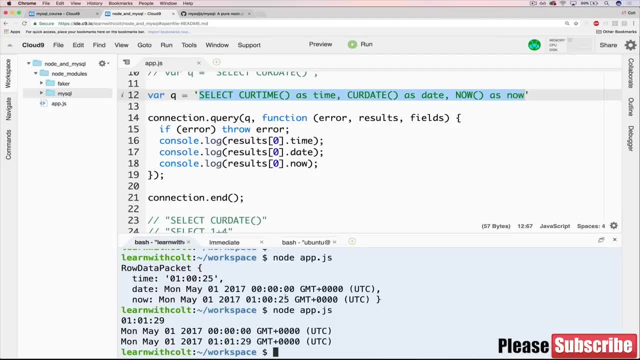 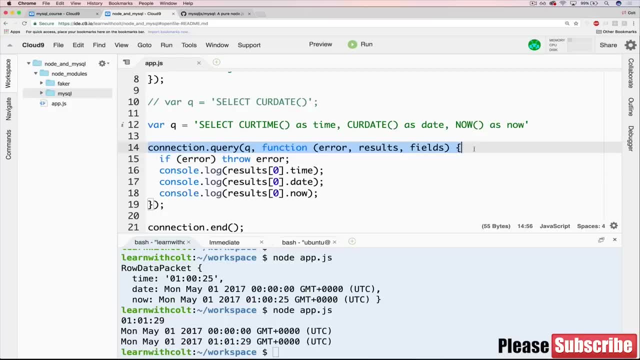 Let's add two or three users and then we're going to see if we can fetch them from node. But before we get there, one thing I want to address very briefly is when we're looking at this code- you know this connection: query function- error results. 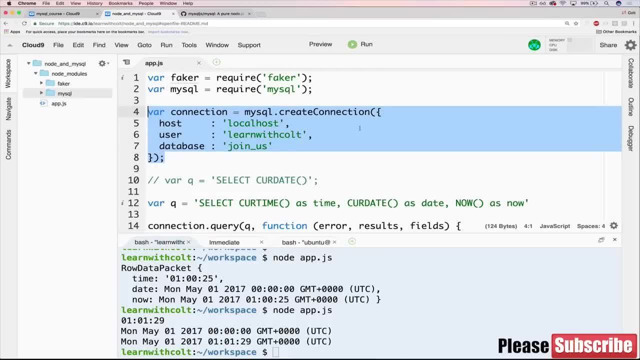 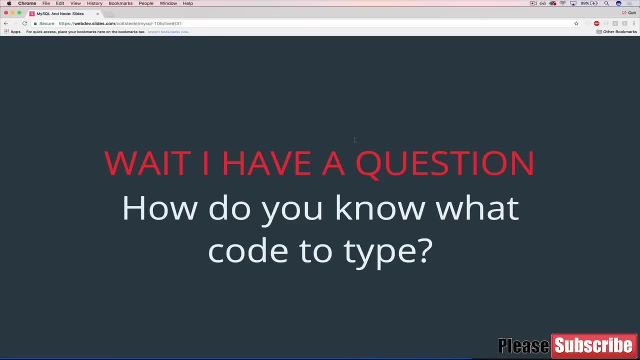 fields, or this code up here for our connection equals blah blah, blah, blah blah. You might be wondering: how did you know what code to type? Where did I find this? It's not in the MySQL documentation. This is not an official MySQL sanctioned library. 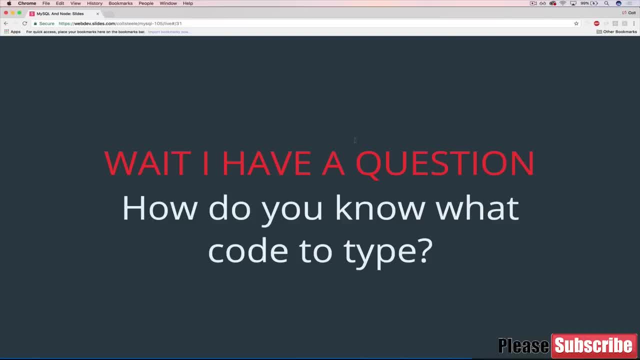 Basically, the way that it works is that random developers, teams of developers, solo developers- go and create these libraries that connect MySQL to other languages. Some of them are more supportive than others. Like I said, some of them are just one person, but they usually have their own documentation. 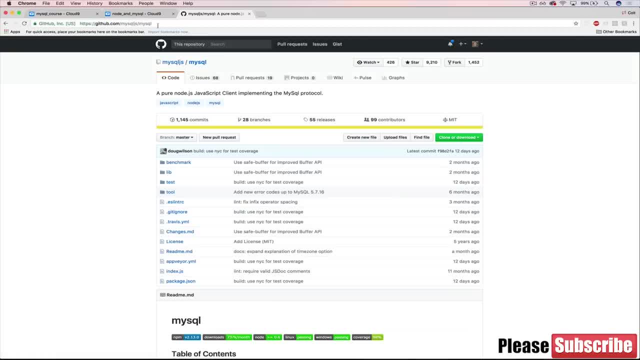 So the documentation for this is on GitHub. It's githubcom- slash- MySQLJS, slash MySQL. There goes my fridge again. Oh, very active today, But if we scroll down you can see: well, there's a lot of stuff to take a look at. 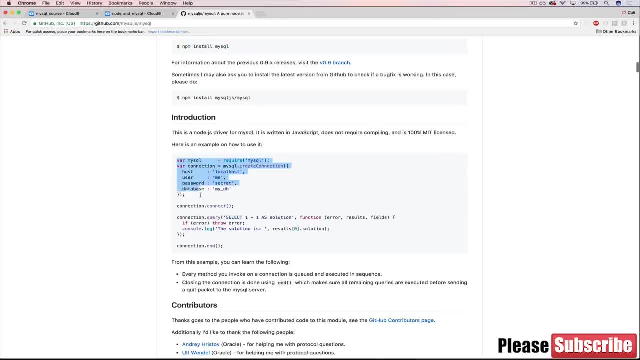 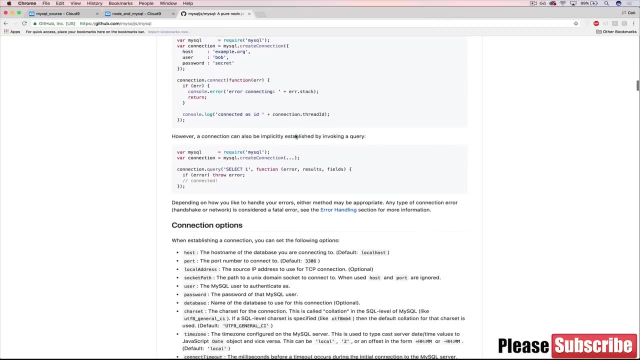 But it basically talks about installing. it talks about setting up your connection. It talks then, if you keep going down about, once you've established a connection, what can you do? Well, here's a very simple query. We saw something very similar, although. 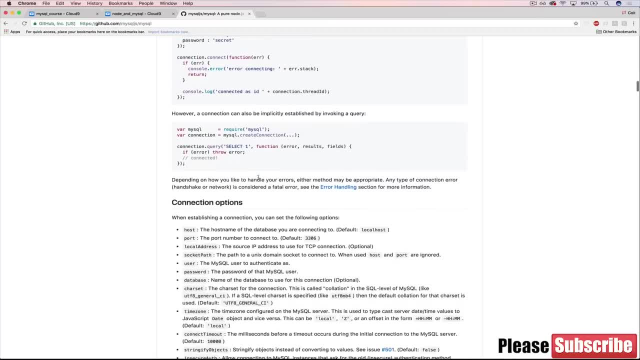 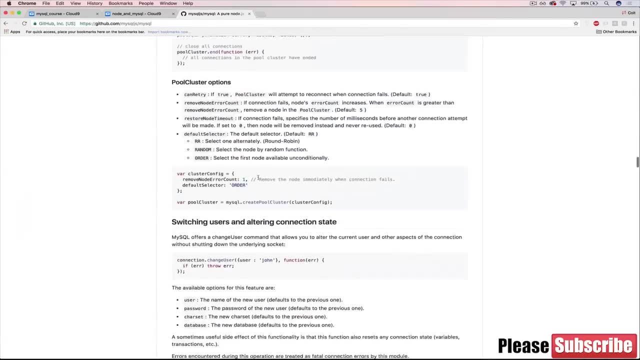 this is just selecting one. We did something a little more complicated, But if we keep going, eventually you'll see we get to things about querying, which is where we're going just in a little bit. But basically I want to show you there is a source of documentation. 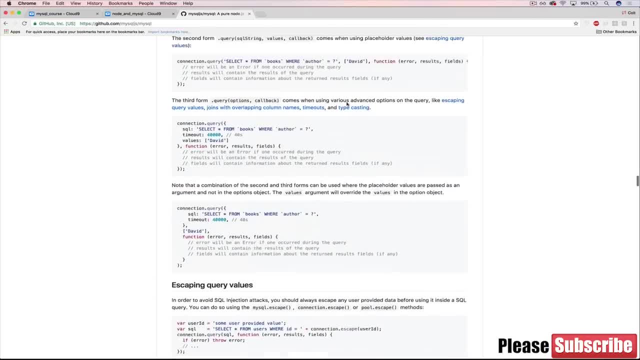 So here we talk about some queries how it works. We'll come, we'll come back to this in a bit. But I'm not just pulling this stuff from nowhere And I certainly don't have it memorized. I'm not just, you know, I don't just know how it works. 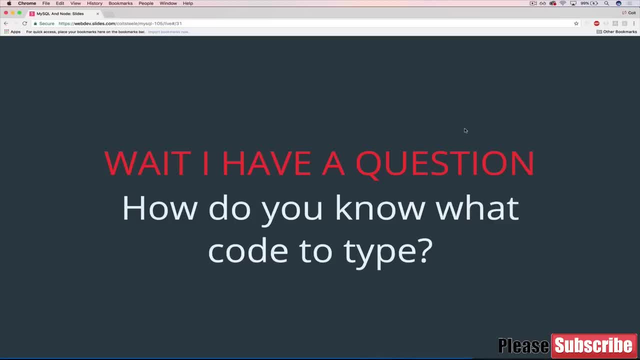 I'd say the approach is more OK. I know what I need to build. I'm going to be building it with Ruby. Now let me find the Ruby MySQL driver, or a gem, which is what they're called, instead of packages in Ruby. 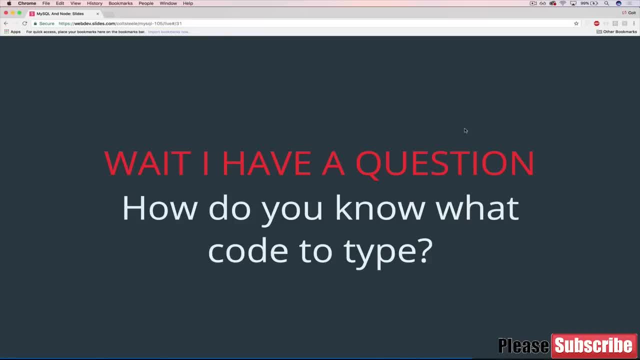 Let me find the MySQL gem. Is there a connector? And then you find it, And then you look through the documentation and you figure out how it works. OK, how do I connect first? That's the first thing you need to do. 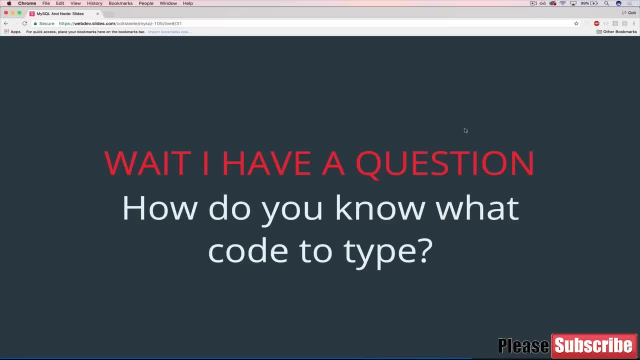 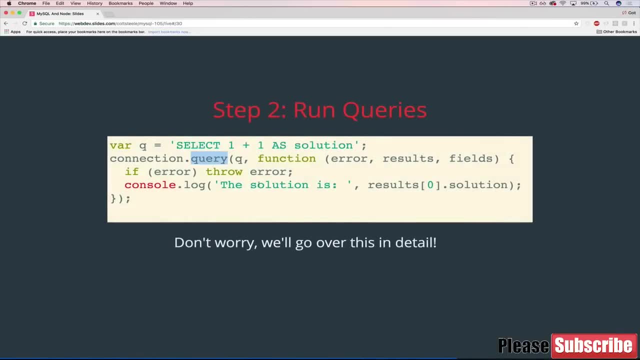 And there's not one syntax. It varies from language to language. Somebody made a decision. So if we go back to our slides here, you know somebody made the decision to call this method query, Which I mean it makes sense to call it query. 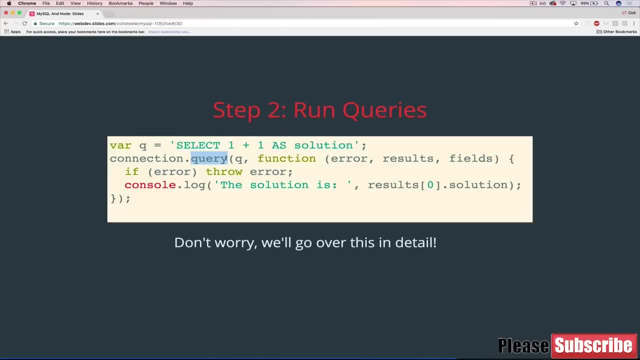 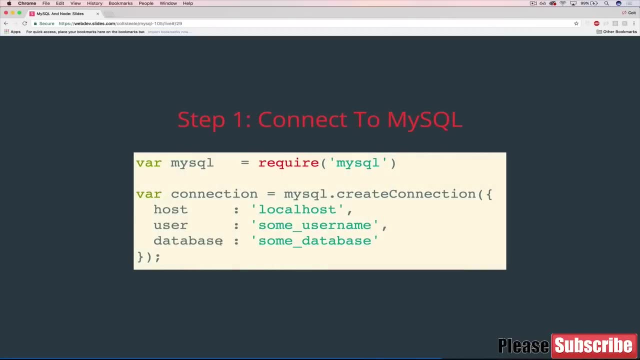 but it could have also been called make query or perform query, Or when we're creating a connection, MySQL dot create connection. I don't know. Someone could have called this. This could be database name instead of database, But somebody is making those calls. 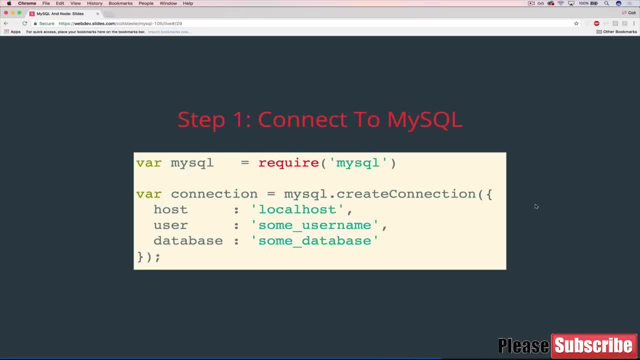 And I'm not disagreeing with the way this is named in any way, But I'm saying you have to play by the rules of whoever defined this. Just like when we're working with MySQL, we have to use the MySQL syntax. There's a specific syntax we have to learn. 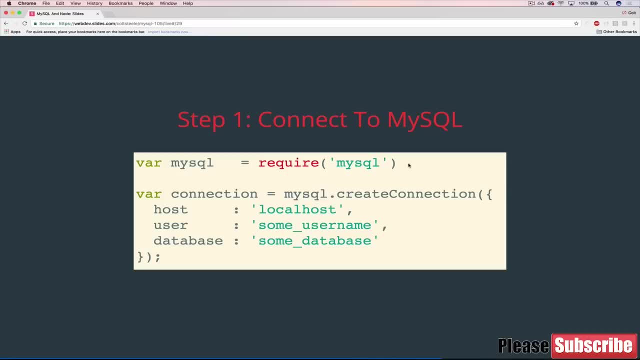 Same thing for using these libraries. So it's not something that comes standard with JavaScript or with Node. It's something we had to plug in ourselves, And that means we need to go do the work to figure out how to use it. OK, so next up, we're going to create our schema. 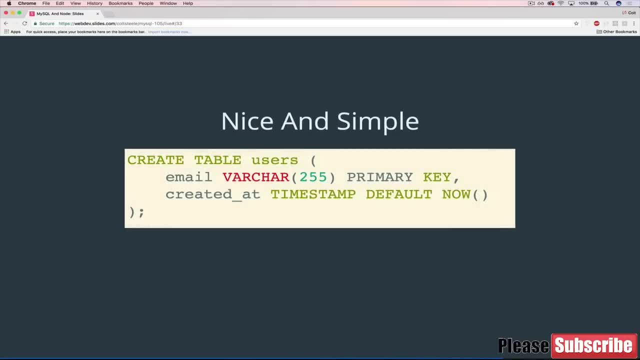 And it's pretty simple. All that we need are two fields. So we'll run, create table users, We'll do email and a pretty standard length is two hundred fifty five. So not that an email is that long, But for fields in general, text fields, people will do varchar two five five. 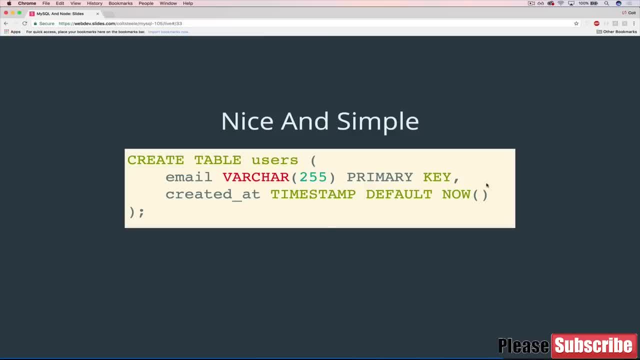 and we'll make it a primary key. Why do we want to do that? Basically, we don't want someone to be able to sign up twice with the same email address. Also, it gives us a couple more options for exercises, so it's a good thing to do and it's good practice. 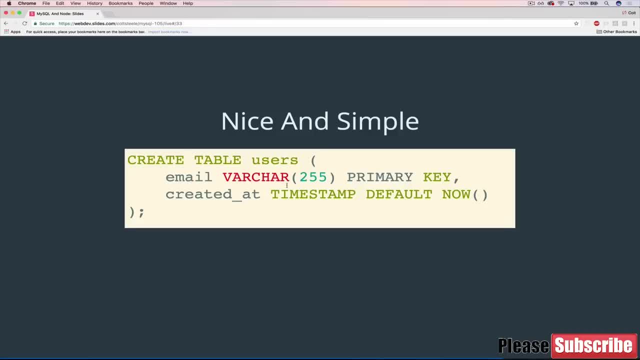 This is probably the first time we've seen primary key without auto increment. Then we've also got created at And that's going to be a timestamp. It could be a date time, but remember back to that video I did about the difference. 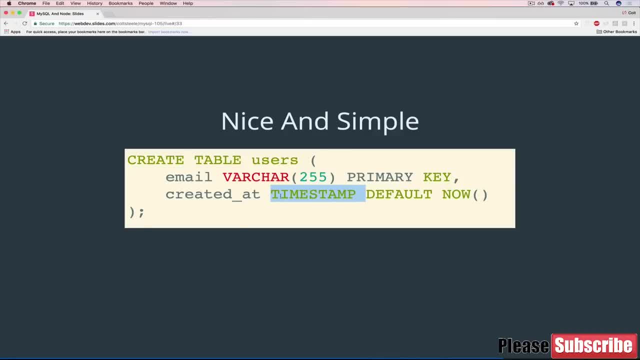 Timestamp is smaller, It takes up less space and memory and it works just as well, except for really far away dates in the past and in the future. Nineteen, seventy up until twenty, thirty eight, I think it is, is the current range. 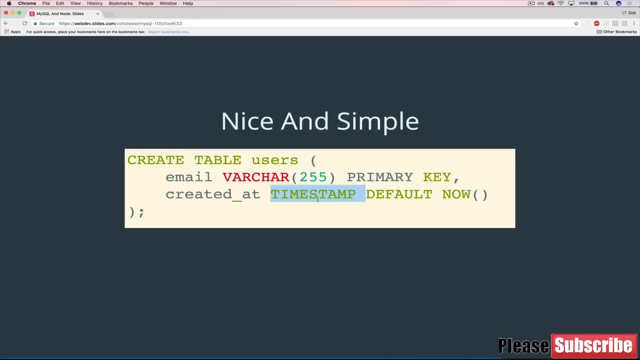 We're not going to worry about that, because we're dealing with current dates. We're creating a mailing list app or a waitlist app. People are signing up now, so we don't Nobody's entering a date from 1650 or something. 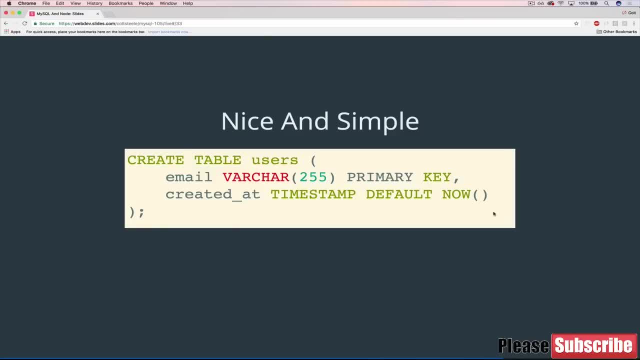 Then we're setting the default value to be now, so that when someone signs up, it will automatically be filled in as the current time. But don't forget, when we're working with Faker, we are going to insert like 500 users into this table and we are going to provide a created at time so that we 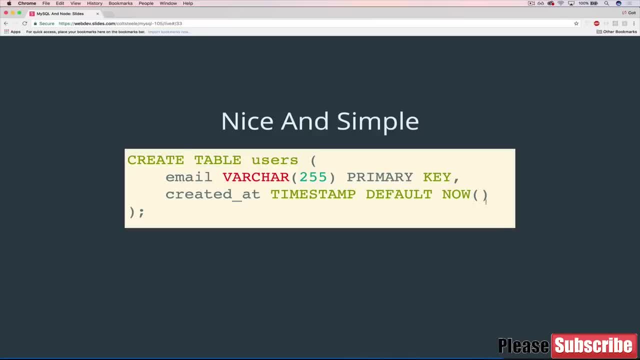 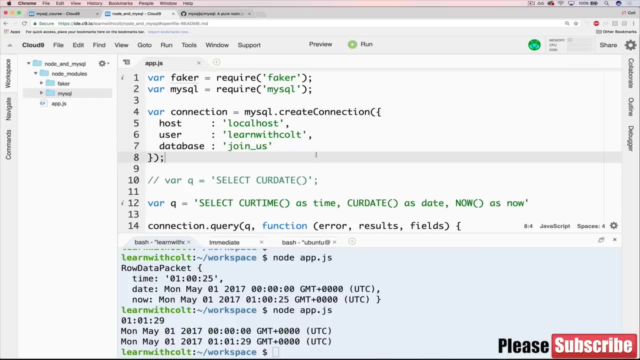 don't get 500 users with the exact same time, So we want this default value to be there, but we'll also be able to override it manually if we want to. OK, Let's hop over to cloud nine, And the first thing I'm going to do- 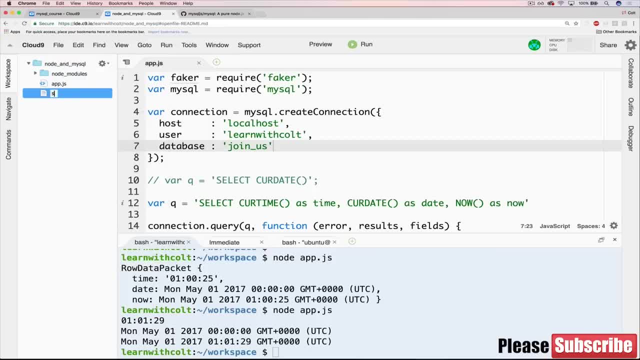 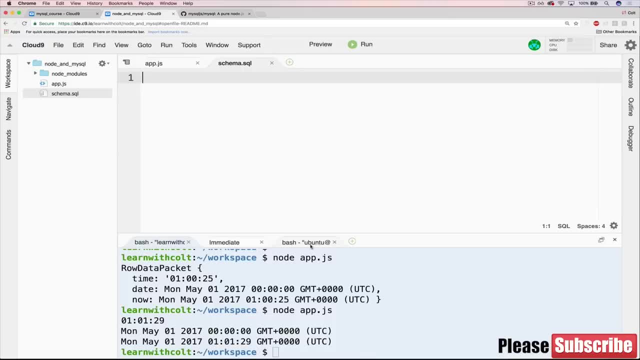 close this down is just make a new file. I'm just going to call it schema dot SQL, And the only reason I'm doing that is just to have a record of this. You could just open up my SQL and start typing: create table. 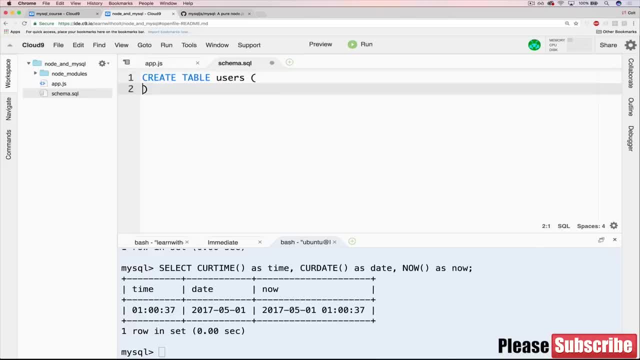 I'm going to do it in here: Create table users. OK, so we wanted email, and then we wanted: created at an email is Varchar Two, five, five primary key and created at is timestamp would work just fine if you left it as a date time. 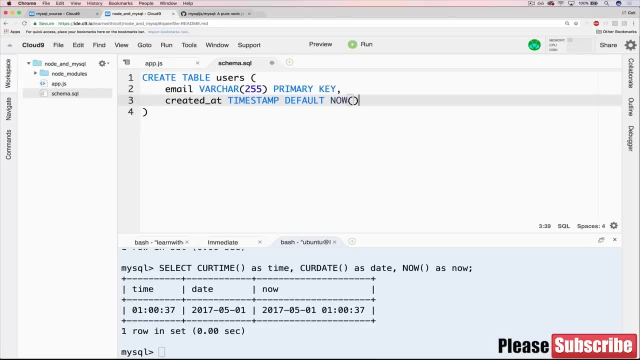 And we want default to be now, or we could also say current timestamp. OK, just like that, And we'll save. We'll hop down to our terminal down here. I'm in the MySQL CLI and I'm just going to select database right now and see what. 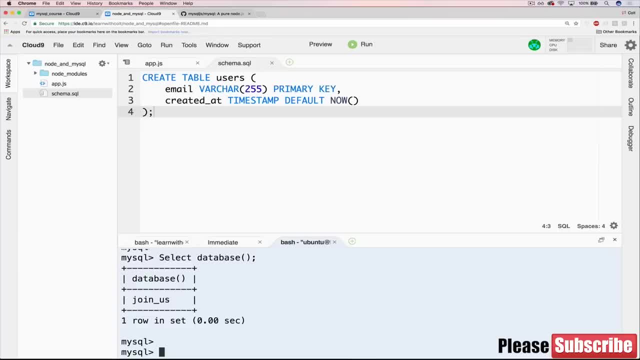 we're working with Good, So we're in the join us database. So we made a new empty database. If we look at, you know, show tables, There's nothing here. That's good. So we're going to create this. 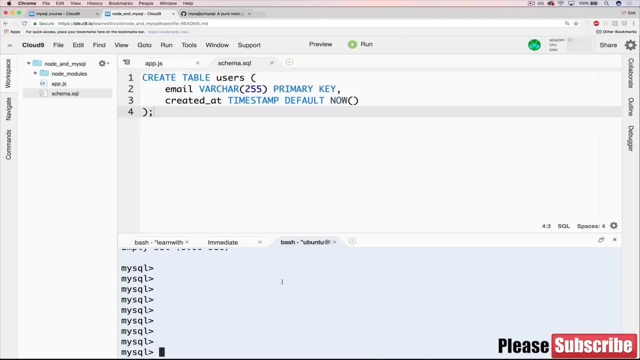 You can either copy it and paste it in, or you can run the file, which I'll do just because it's been a while. source: schema dot SQL. OK, now let's see if it works. Show tables this time. Now we have a user's table and we can describe it. 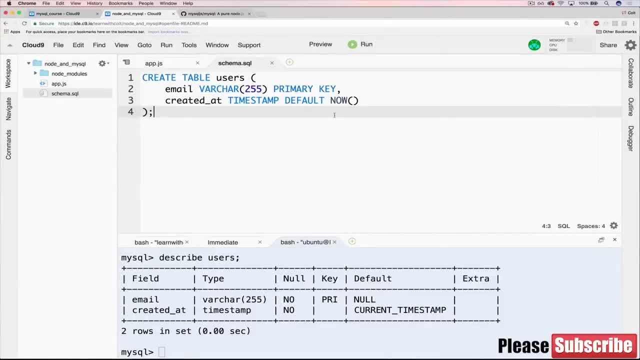 Perfect. So that's all in there, which is great. Now what we want to do is insert, let's say, just two users, just so that we have something. So we'll do an insert into users. This will be one of the last times we're actually inserting stuff manually, rather. 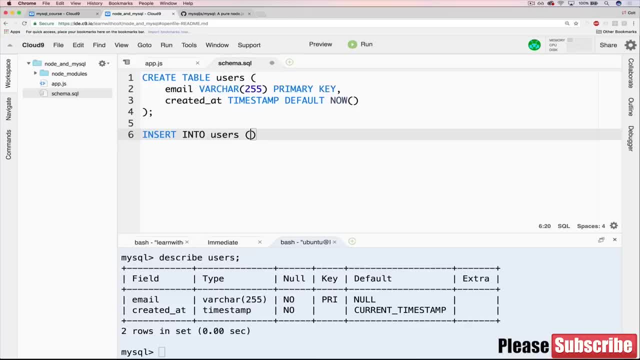 than using our code to do it for us and inserting 500 at a time. So all we're going to do is insert email and we'll leave off created at. for now, We'll just have it be the default, So that means we'll have. what do we want to do? 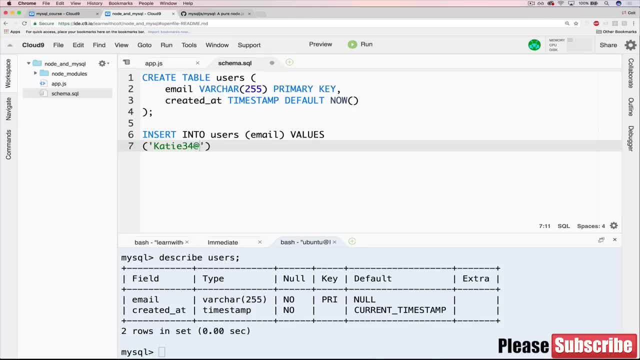 Let's do Katie, three, four at Yahoo dot com, And then we'll add in another one which will be: let's do June Day at Gmail dot com. Sure, Just like that. So just two users. I'm not going to source this again, unless I commented this out. 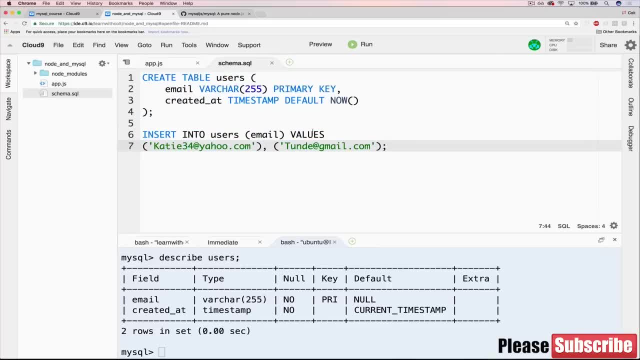 Otherwise it would try and create users again. Just copy this: Do we have any syntax issues? We'll see. OK, it looks good. You can do a quick select star from users. There we go. OK, so we have data in here. 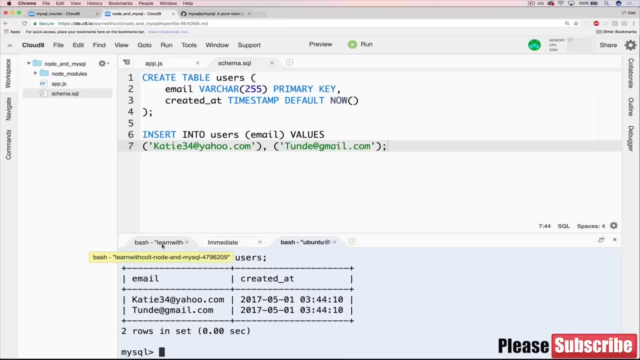 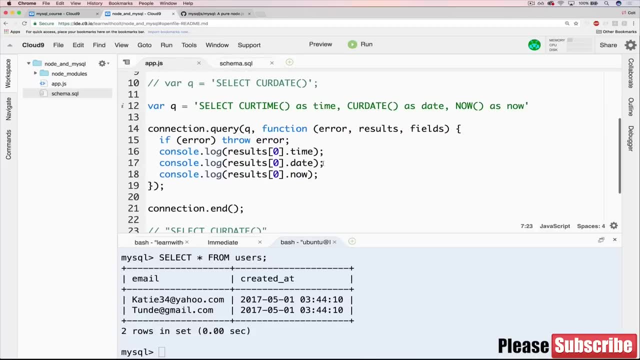 That's all we need to start Now. our goal is to come over to this file and, rather than doing these silly, select curr time and curr date. now we're going to try and select from the users table. We want to make sure that not only are we, 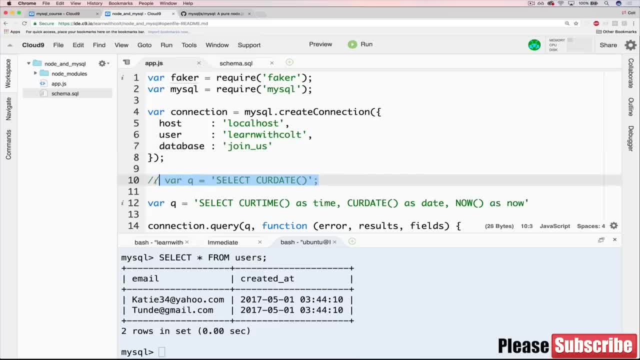 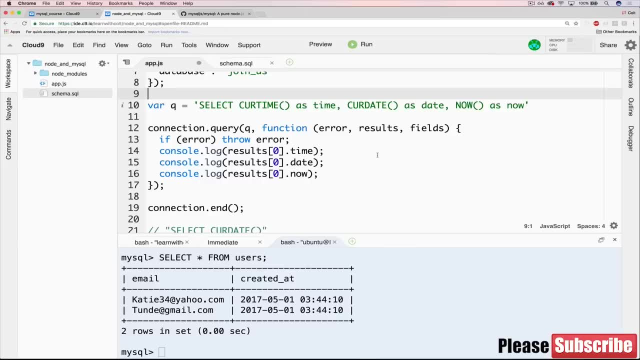 connecting to the database which we've already established. but we want to see if we are able to connect with that table and query it, And the syntax is actually the same. So I have a slide on it. But if you notice, we're just doing connection query. 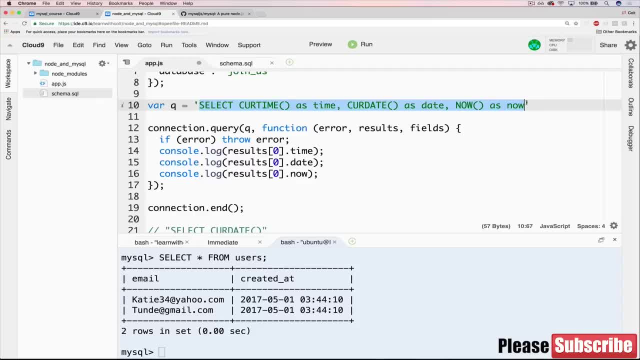 And then we just have a query here that we can replace with whatever we want. So our query is what? How do we select everything from users? Well, we just did it: select star from users. So we'll save that, And you know again, you could just copy it and paste that right there. 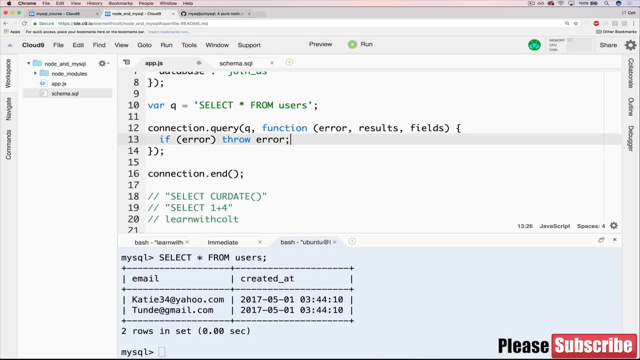 I'm going to get rid of all this because we're not working with time, date and now anymore. All I'm going to do is say, if there's an error, throw the error, And then we'll do console dot log results, just like that. 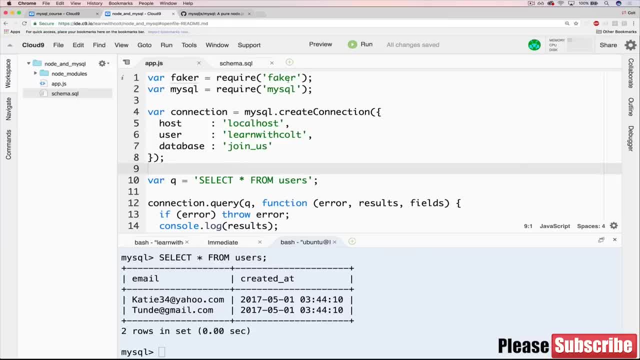 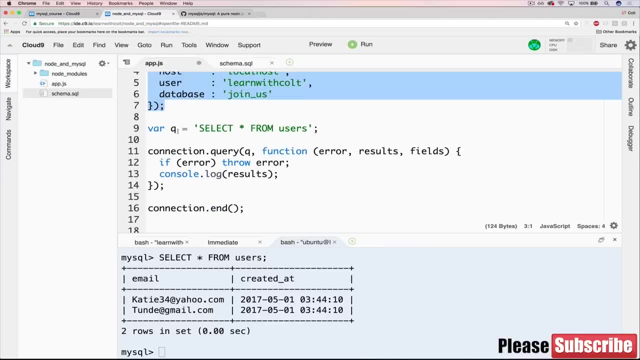 So I'm going to get rid of everything else here, just these. So this is just set up. We're not even using faker can get rid of that. All that I'm doing connecting to the database. Then I have You, which is just storing our simple select star from users. 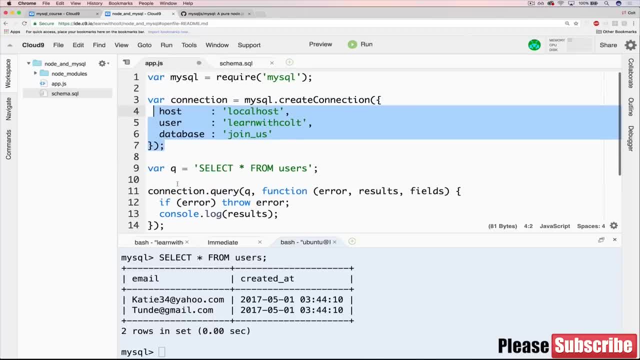 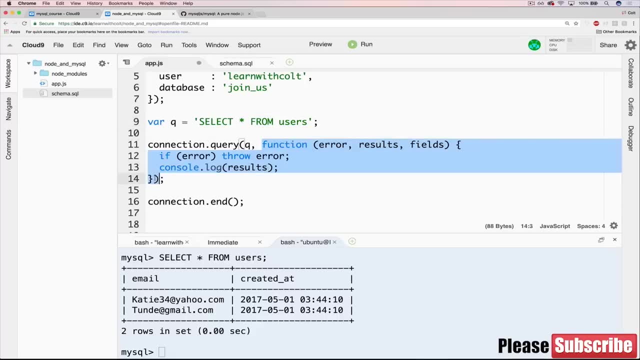 Then I'm doing connection dot query. So take this connection we set up, Run this query, which the first argument is select star from users. The second argument is everything. Basically, it's a function that will be called when our query finishes. 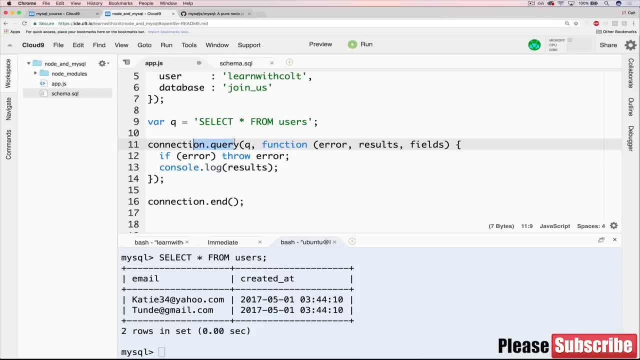 So when it either comes back saying great, it worked, or it comes back saying hey, your database isn't running or I can't find that table, whatever it is, If there's an error, throw the error. If there is no error, this is empty. 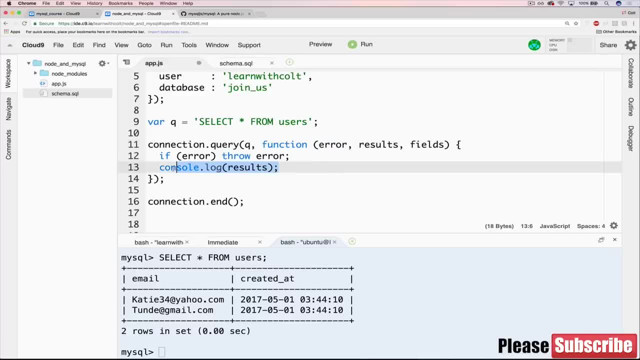 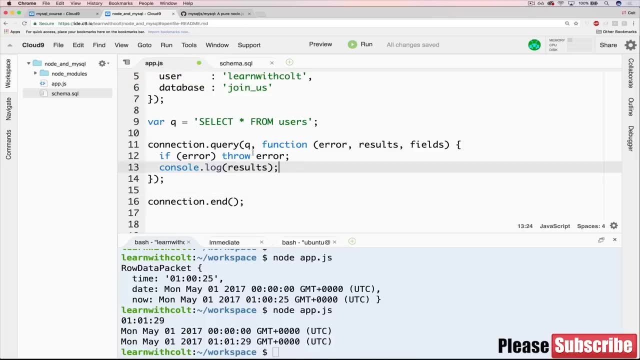 There will be nothing there and console dot log results. So we need to go over to the correct terminal and run it. Make sure we save. I have a circle up there, So save node app dot JS. Okay, Take a look at that. 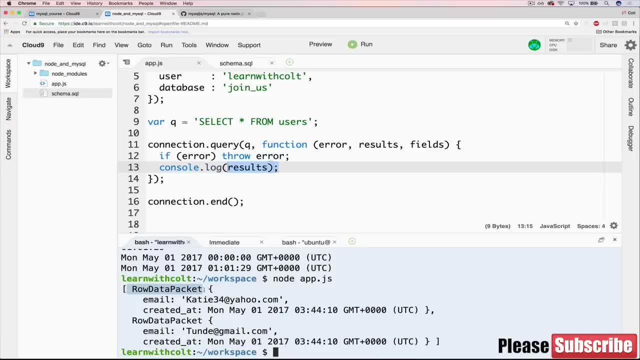 We've got two results. Each one is a row data packet with an email and a created at email and created. So that's looking good, We are getting our data. And if we wanted to only take a look at tune day and his information, 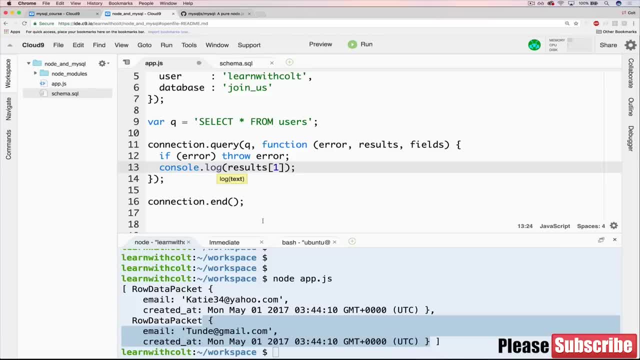 we can drill down and just access results. one their index at zero. It's an array, JavaScript, So this is the zero with result And this is the first save. Run it again. You can see we now are only dealing with tune day. 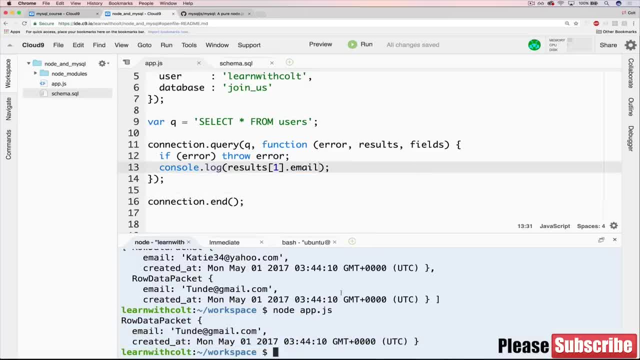 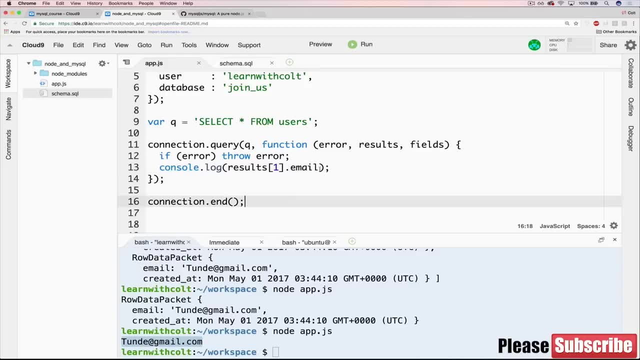 And if we only wanted to print out, let's say, his email, you can just do dot email And there we go. Toonday at gmailcom, Okay, So that's the first and most basic thing that we can do as far as selecting. 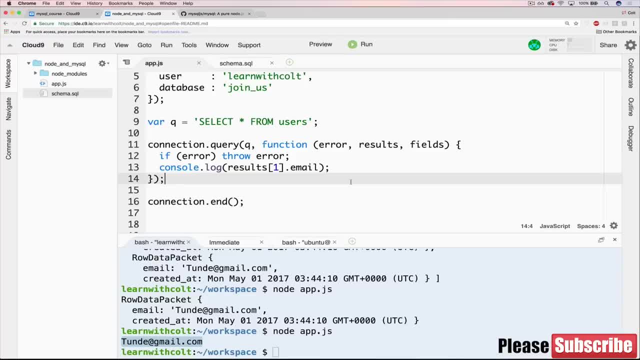 So now, when we're talking about this join us application that we're making, we're never actually selecting all the user information. We're going to have 500 or 1000 users, ideally more. We're not selecting all of them. What we're trying to display to the user is just how many there are. 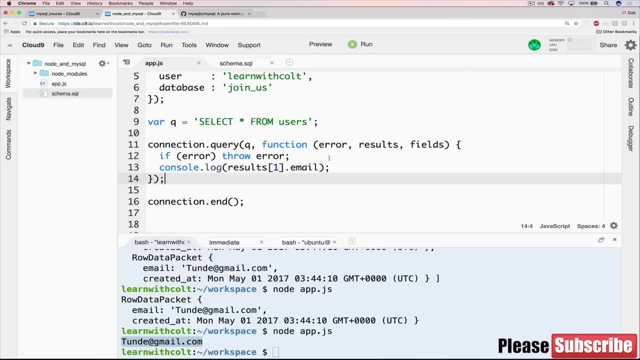 We're trying to display how many users there are, And that is just a matter of counting. Now we could do it a really kind of bad way- I was almost going to curse there- a really bad way, which would be basically select all the users and then just run results. dot length. 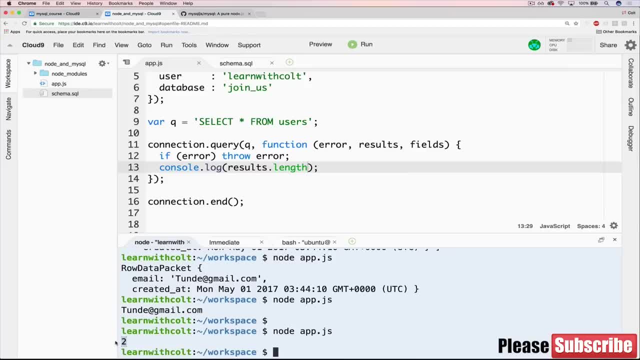 which will tell us how many results there are, which gives us two. So that's a really bad way of doing it, Because if we have 10,000 items in our database, we're going to go select all of them, bring all of them back here, just so that we can do dot length on it. 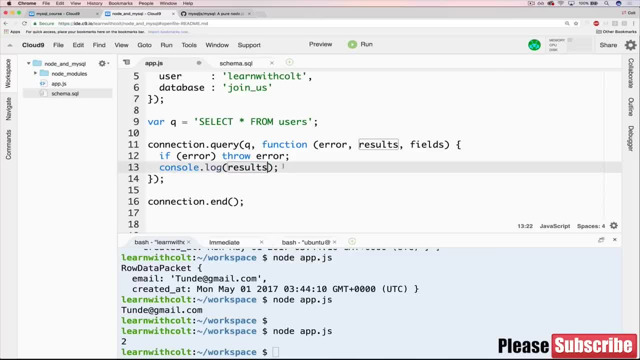 I don't think that's a good way of doing it. So, rather than doing that, what we can do instead is just do count, select, count star from users, just like we've done before Now. if we do it, you can see we get count is two. 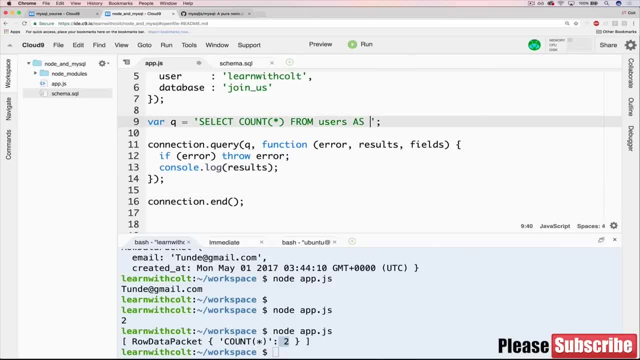 And a nice remember, we can add in an as, so we'll call it as. let's call it total this time, and it needs to go here after the field, before the from, And now, if we run it again, you can see it's stored under total. 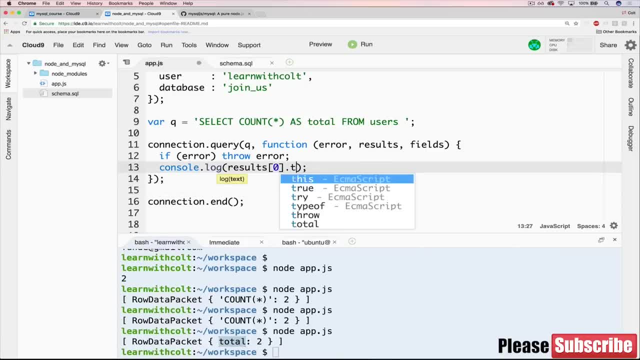 And if we wanted to get that. it's just a matter of results- Zero dot total, Now we get two. So this is a much better way, because we're asking MySQL to count and just give us the count back. we don't actually need every row. 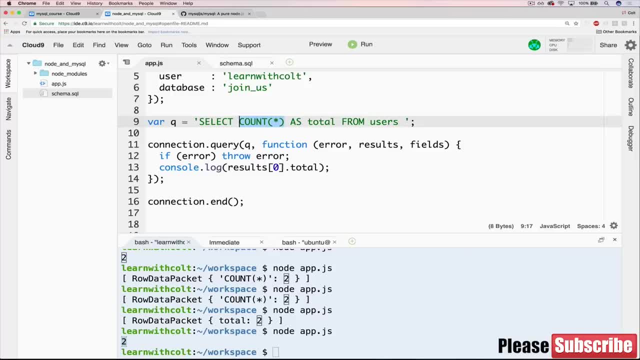 So, instead of 10,000 results back, just give us this count and then we can work with that. So this is what we'll be doing. We will have a query like this when a user goes to the home page of our application. 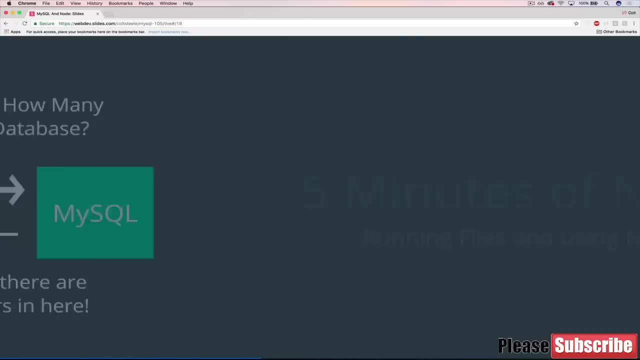 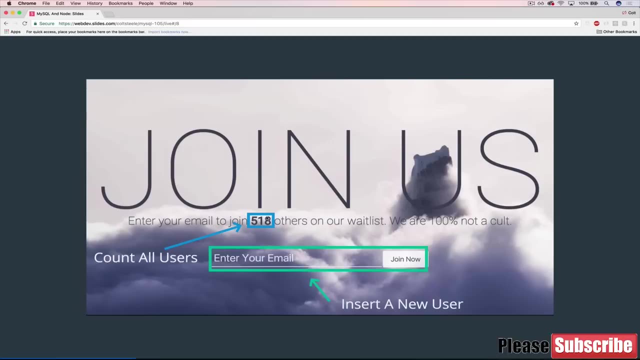 Bear with me while I scroll back. Should probably just edit this. Speed it up. OK, but when a user goes to this page, this number is the result of our node or Nodejs running that connection query, select count, star from users and whatever. 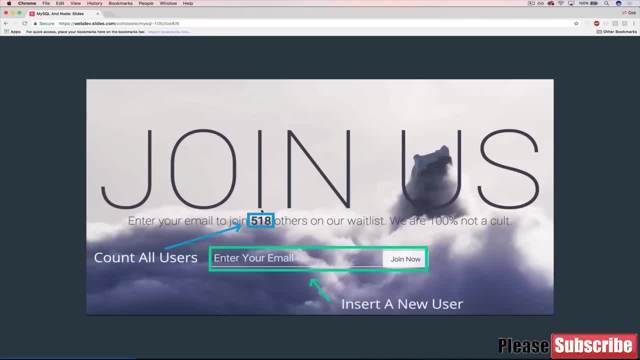 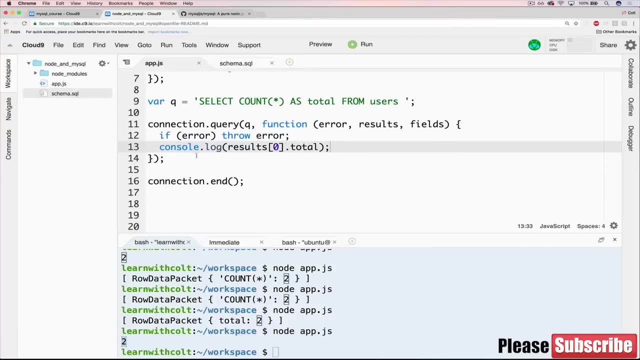 number comes back, we are sticking in the markup in the HTML. OK, so then that brings us to inserting data. What if I wanted to instead insert a new user? So I'm going to copy this. Well, first I'm going to comment that out. 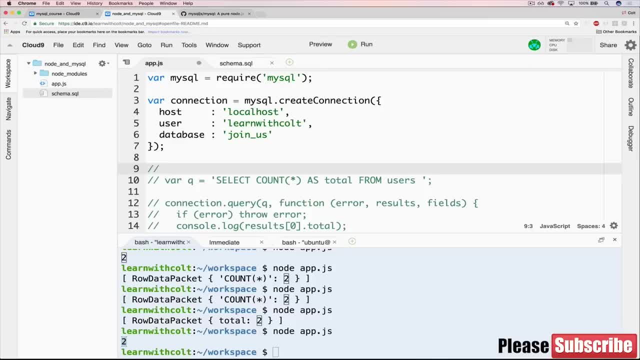 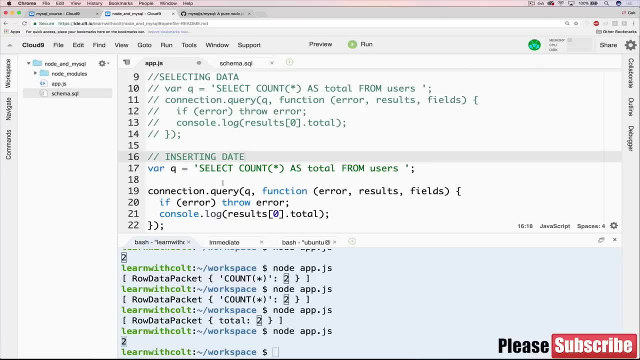 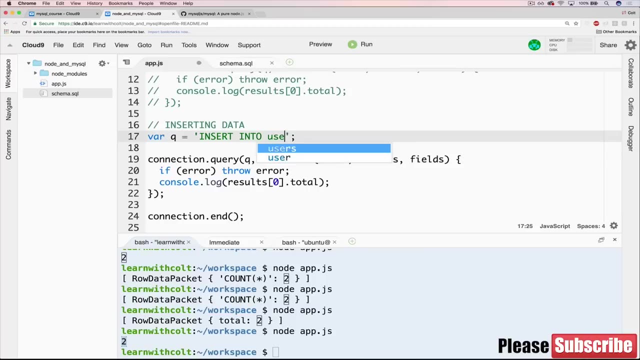 So we have a record of it And I'll make a note Selecting data. OK, now we're going to try inserting data, And you would think that all we needed to do something like insert into users, specify, let's say, email. 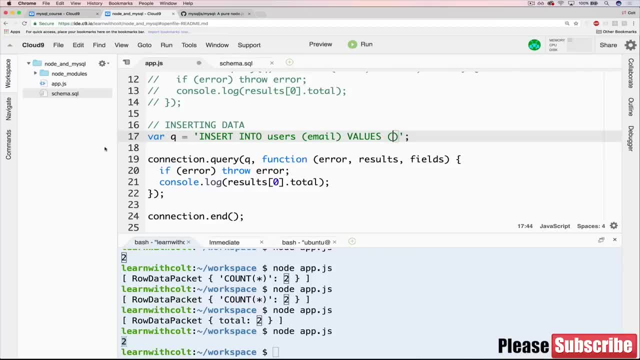 values, and then all we want is: we'll do one here and we have to pay attention to quotes, because we're working inside of a string. We need to use double quotes here. And let's say we just make up an email, We'll call it Wyatt. 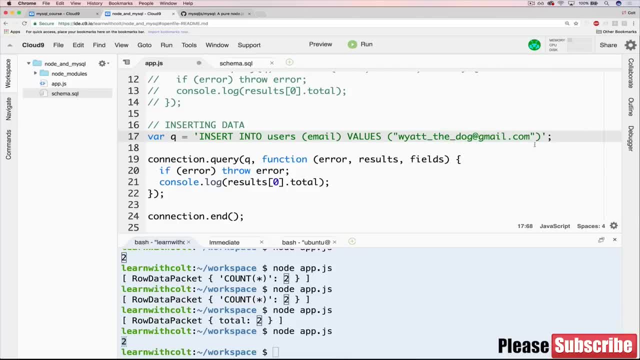 The dog at Gmail dot com. it's one of my family dogs. So if we do that and we insert that, So if we kept everything else the same, let's just console dot log results, just like that, And if there's an error, throw the error. 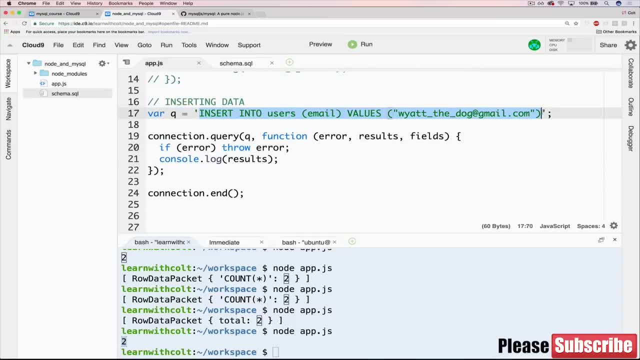 So this is regular SQL, right? If we ran this and we could verify it, of course, If we ran this right now, it works. So now let's change this a little bit so that we don't end up with two of them. 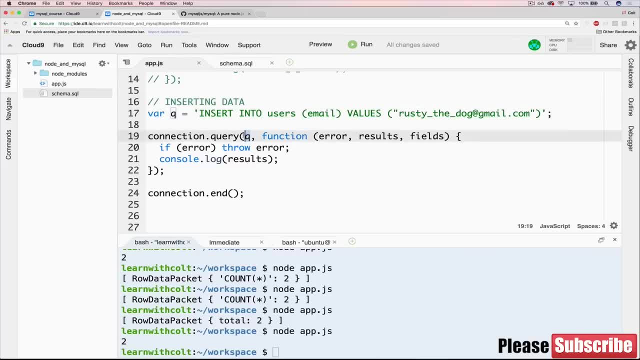 But everything else is valid. So let's do that, Run it. Connection query: This query function, blah blah, blah, blah, blah. If there's an error let us know, Otherwise print the results. Let's see what happens. 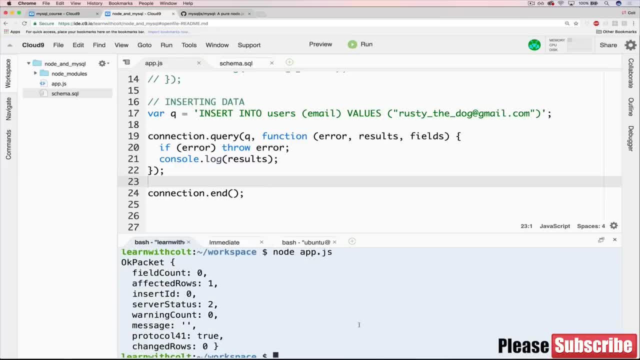 Okay. so look at what we get back. First of all, it says: okay, packet, we get field count zero. Affected rows is one. There's no message. Everything looks okay If we went over here and did a select star from users. 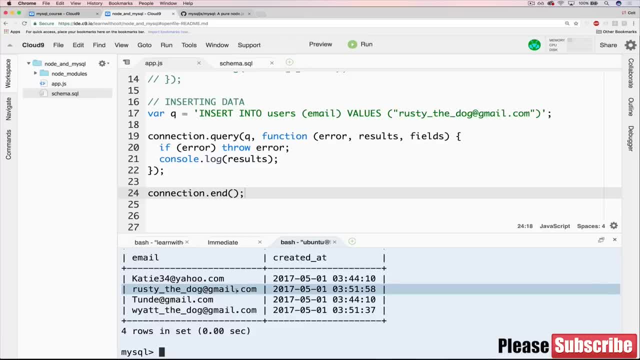 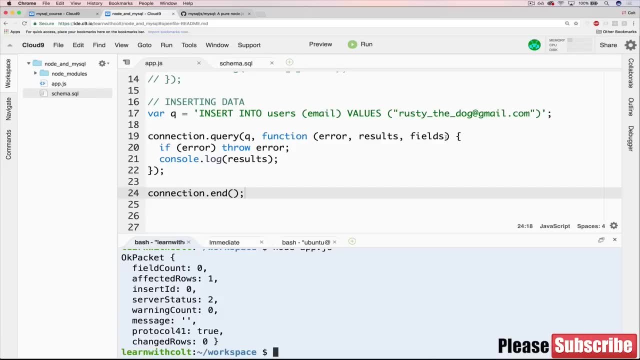 you'd see that Rusty the dog is now in here, So all of that is looking good And that's correct. This is working how it should work, which is good, But this is not something that really is helpful to us, Inserting one item at a time that we're 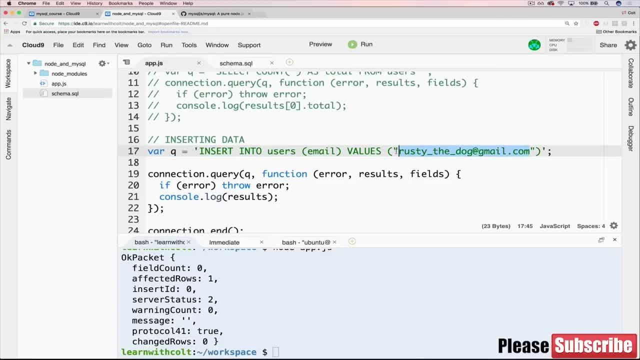 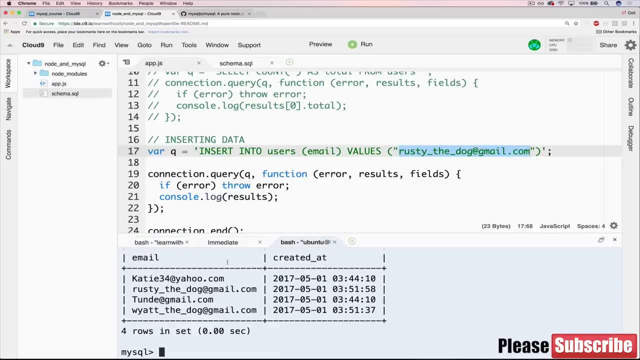 hard coding in where I'm saying Rusty the dog. that's just not great. Like this is SQL we're writing. If we wanted to insert Rusty the dog exactly, we could just copy it and do what we did and paste it here. 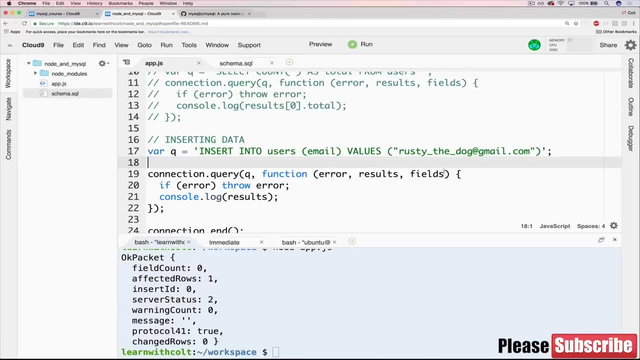 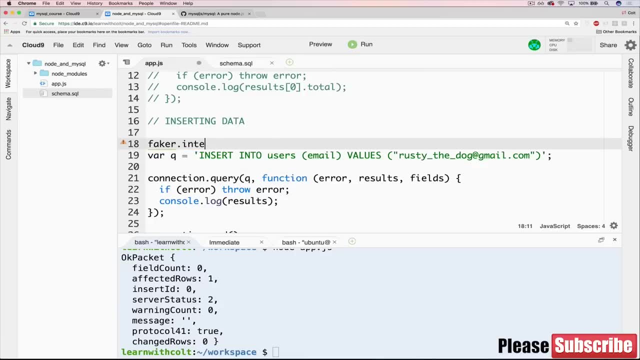 What we want is to be able to do dynamic data. So I want to be able to say which we don't have Faker set up. but I want to be able to say: Faker dot Internet, dot email, which is going to give me a random email address. 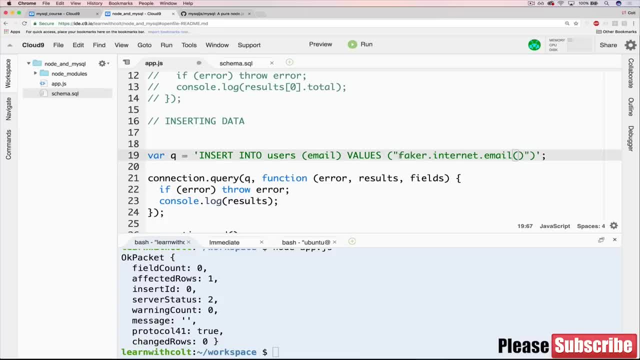 And I can't just stick that in here. That's not going to work because it's going to just try and insert an email address: Faker dot Internet, dot email. So there's another syntax we use. In truth, you'll probably never use this. 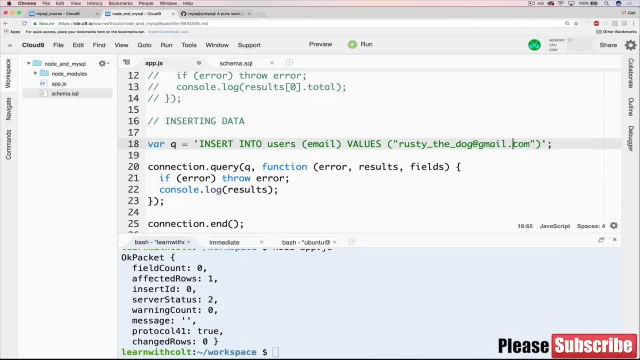 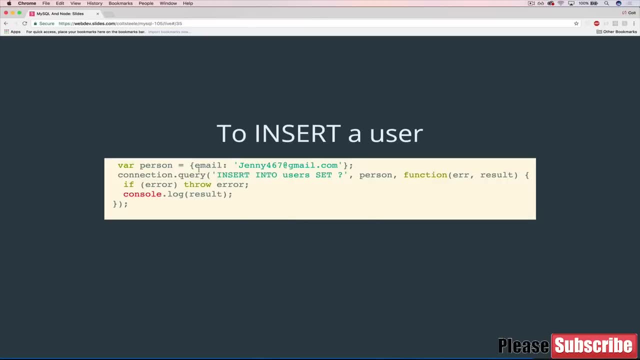 for inserting where you're actually hard coding. in the data you're trying to insert. What you'll actually do looks something like this. So we have a slightly different syntax. First thing you'll notice is that I'm creating a variable that is storing the person of the user we're inserting. 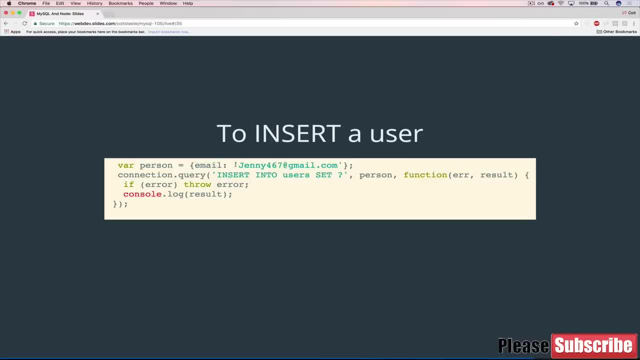 And it's a JavaScript object where I have a key email and then a value- Jenny, four, six, seven- at Gmail dot com. We'll come back to that. Then our connection query looks the same, but our query is different. We're doing insert into users and then this weird set question mark thing. 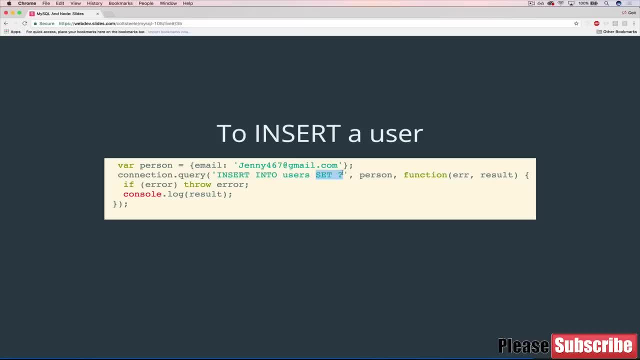 We've never seen that. Is that valid sequel? This is something else. And then also we have a new argument. We're passing person in as well, And then our regular function with error and result. So what I'm going to do is copy this over. 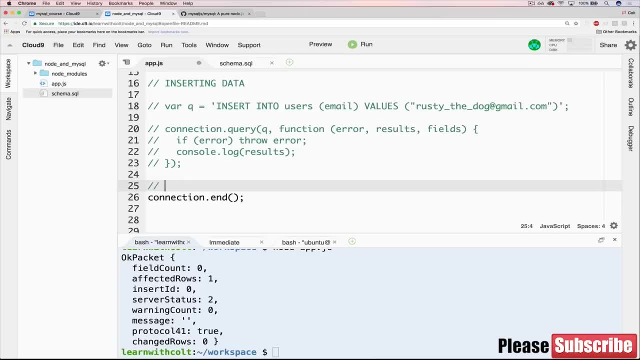 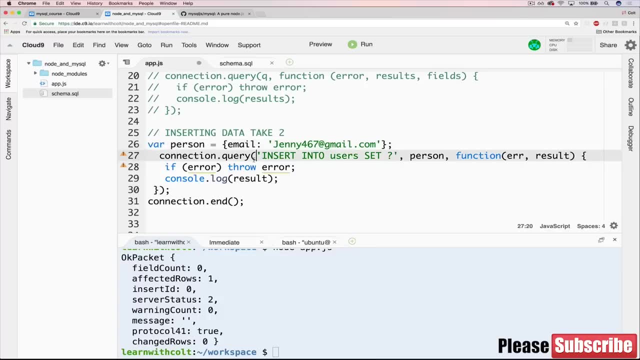 I'm going to comment This one out as well, And I'll call this inserting data. take two and paste this. OK, so a couple of things to go over. One: does it work? We'll try that in just a moment. 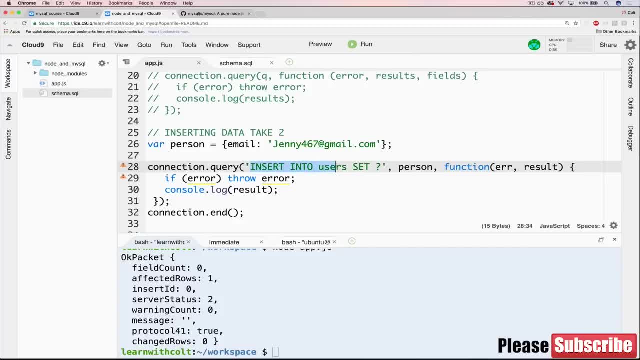 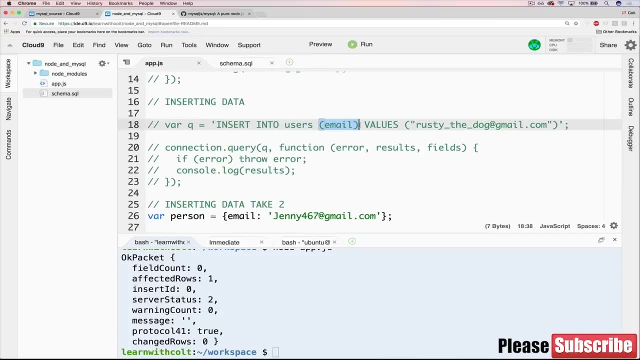 And two: how does it work? So we've got this insert into users. That's the same right. That's what we had up here: Insert into users. But then we had to specify exactly what we're inserting. So we'd say email. 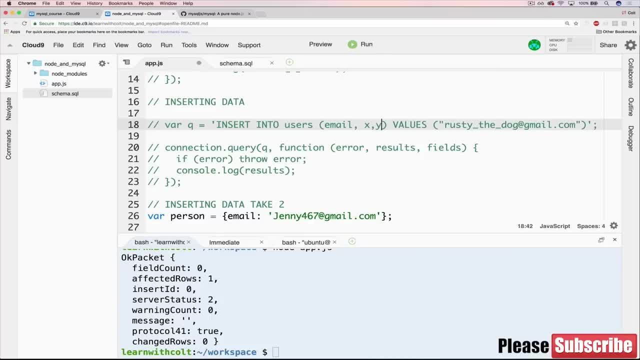 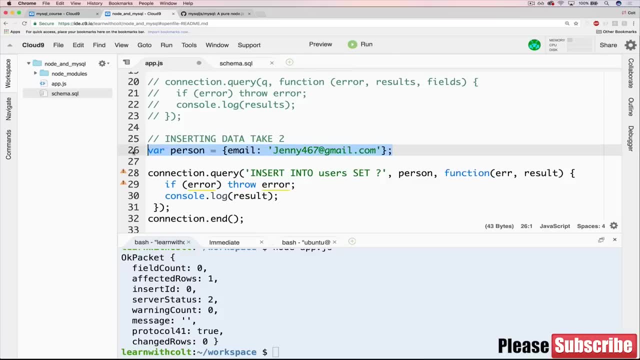 And if we had ten columns, we'd have to say email, comma x, comma y, whatever they are right, as we're used to. But there's another way. What we can do instead is make a separate entity in JavaScript. 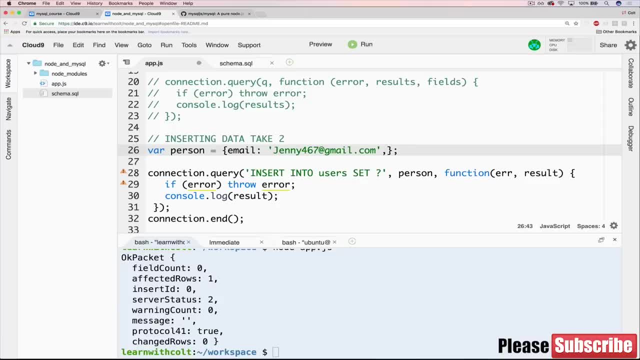 an object where I could come in here and do something like email is Jenny. We don't have name, but we could have if we had it in our database we could have. name is Jenny. we could have 20 different things And to insert it all correctly, all I have to do is connection query. 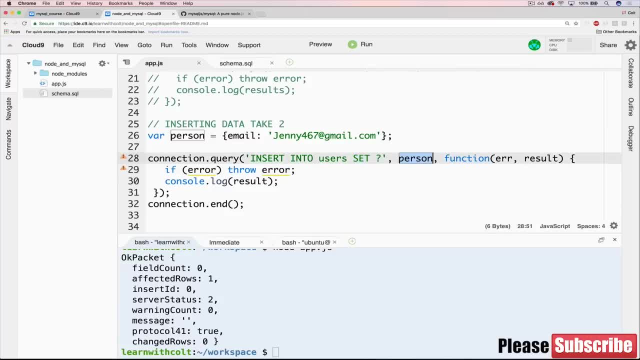 insert into users and I add: set question mark, And then the second Agreement is this object And what will happen? is this MySQL fancy library? this package will basically take this object and then we'll figure out. OK, there's something called email. 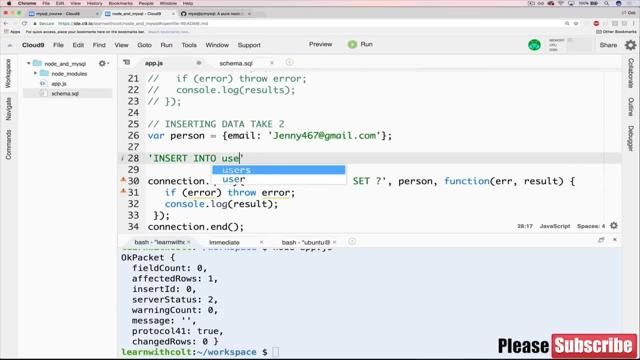 Well then, I'm going to turn this query into insert into users Email Values: Jenny at Jenny. 467 at Gmail dot com. we have a quote issue again, So I'll make this double quotes. OK, so it will turn it into this. 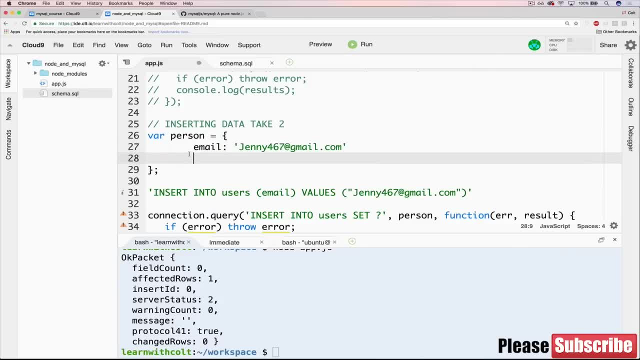 But if I had something like Email- and let me indent this a little bit better- Let's say we had email comma And let's say birthday Is 2001,. comma 11,, comma slash 11.. It actually dashes from MySQL, but let's say we have that. 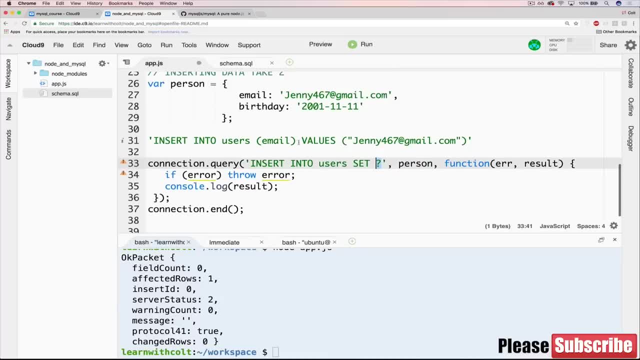 Well, by just passing it in Here, I never have to mention birthday. It will know when inserting it to then have birthday equal to this. So I won't go and type the whole thing, but the point is that it can dynamically do that for us. 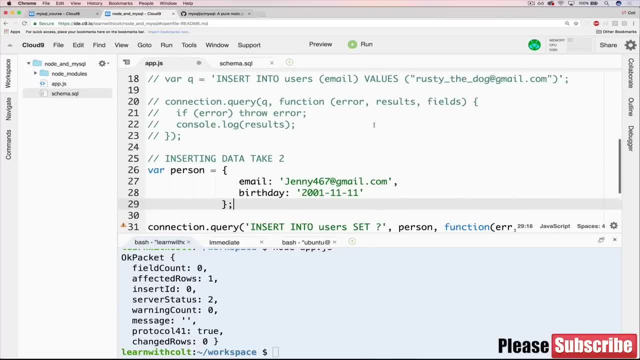 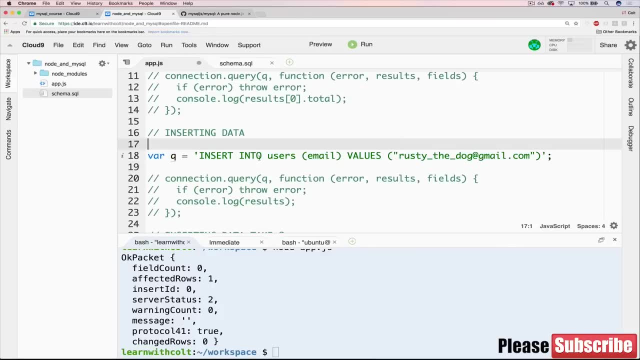 And that doesn't seem that helpful. when we're inserting one thing like this, It's the same problem that it wasn't a problem, The same thing we ran into here, Like if you're just inserting this one hard coded email, Why does it matter? 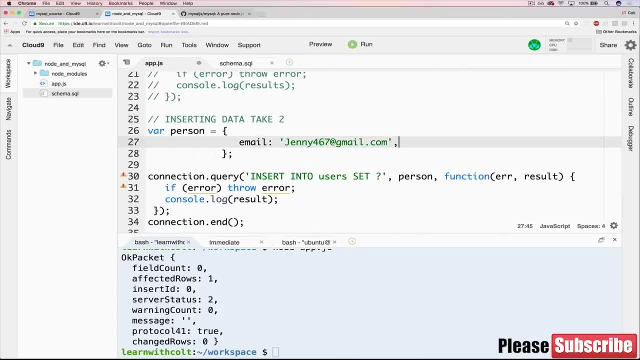 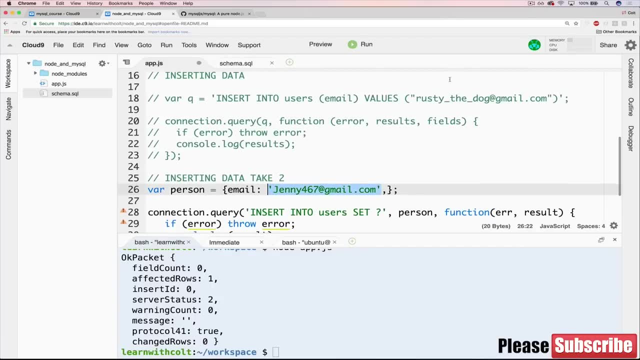 The answer is down here. Well, it matters, because now we don't have to hard code it. What we can do is change this string because we're no longer part of up here. Whatever we're typing is inside this text, But down here it's not. It's separate. 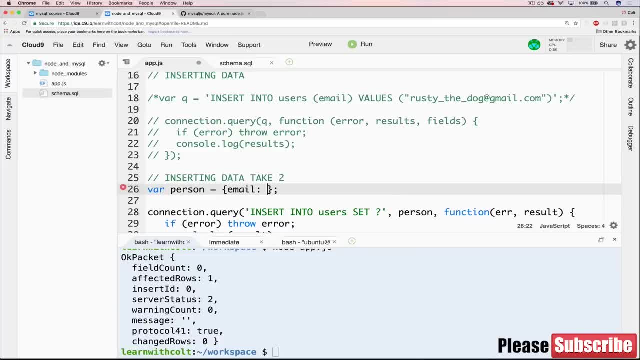 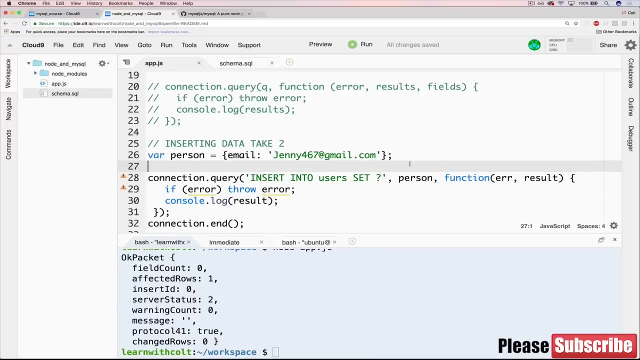 So we can replace this with something dynamic, like using Faker, But let's start by just making sure that Jenny works just like that. Jenny467 at gmailcom. Let's save and let's see what happens now. Insert into user set person is this: 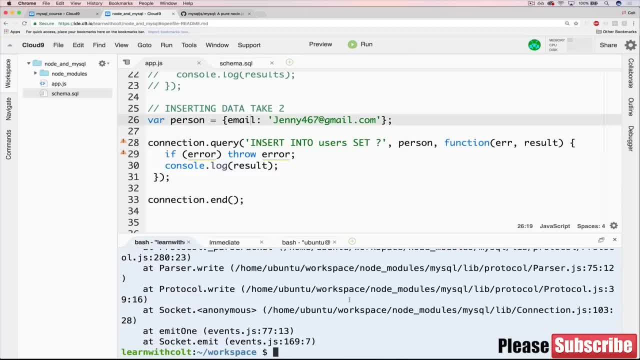 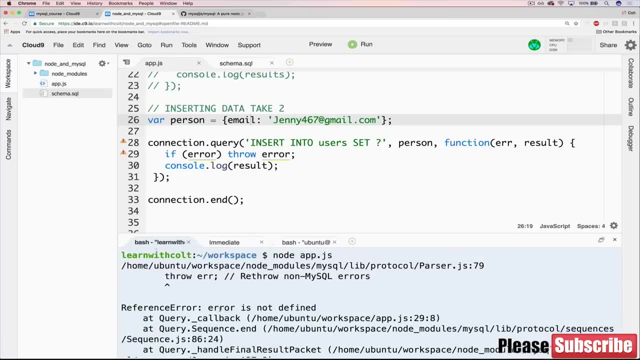 Okay, And it looks like we got an error this time and it tells us: Oh, okay, Well, this is a silly one, This is my fault with the code, but it's something it's good to talk about. If you look at what the error is telling me, error is not defined. 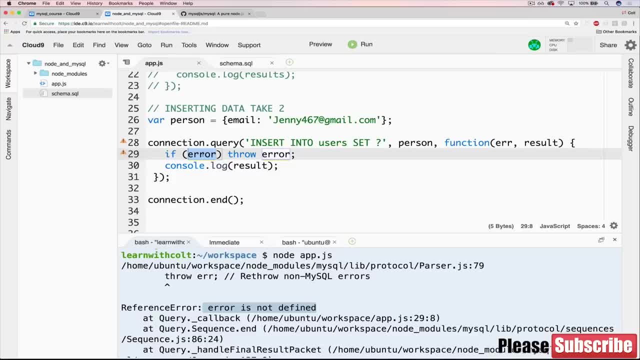 So it's saying this thing: error is not defined. And actually I was ignoring these, but I'm sure Cloud nine is trying to tell me: Yes, it is. It says error is not defined, And that's because up here I called it ERR. 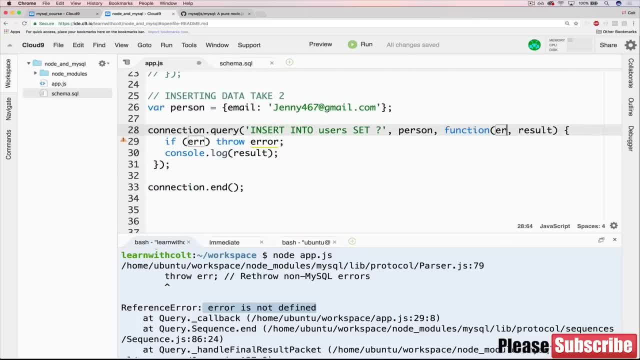 You can call it whatever you want, So I could call this mistake in all caps. It's a bad idea. It would be a mistake to use all caps, but as long as they match, So I'll go with ERR, though That's a standard thing, just like that. 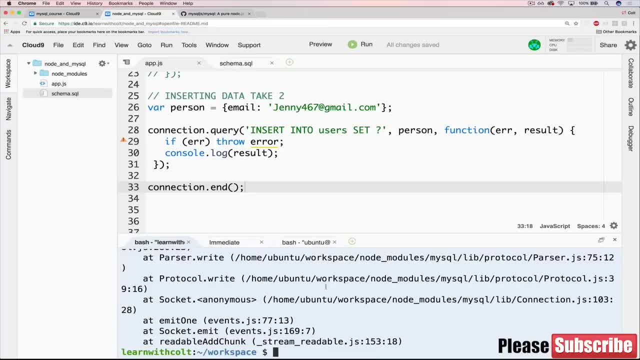 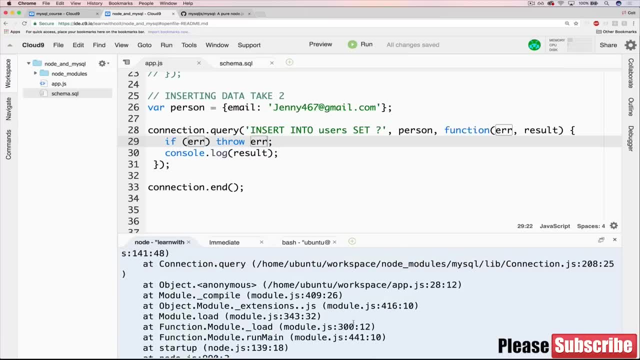 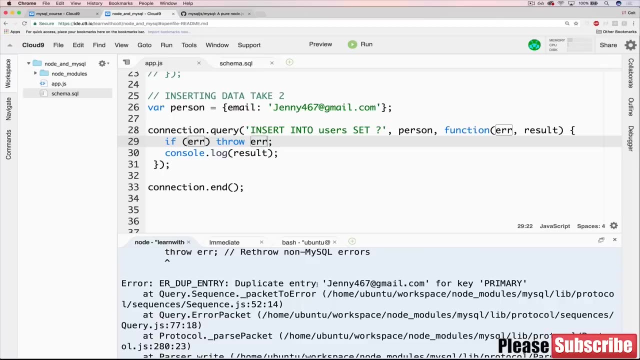 Okay, Now we get a different error this time. Oh, my goodness, It's the same one. Jeez. Now we get a different error. This time it's saying duplicate entry. Great, This is good to know. Now it's telling us we already have someone named Jenny 467 at gmailcom. 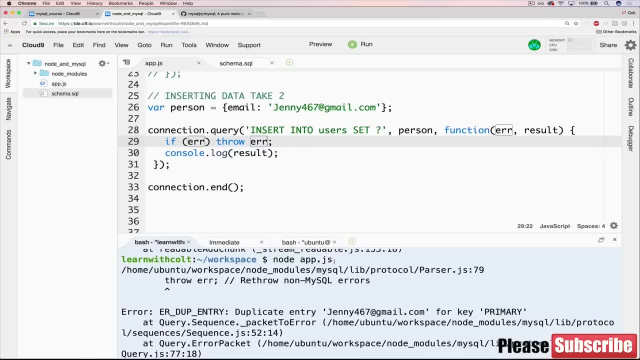 And the reason we're getting this error is that we already have a Jenny in there. So this is interesting And this is why I added that primary key. So we, just like one second ago, inserted Jenny 467 at Gmail And we hit this problem with the error coming back where we had a syntax error. 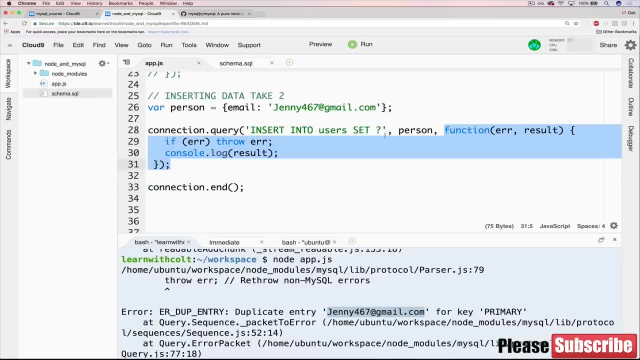 But it was still inserted. Remember, this code only runs when the insert of the query is done. So we inserted Jenny 467.. Then I screwed up our code And so it broke right here, But Jenny was already added. So now we just added another Jenny, or we tried to. 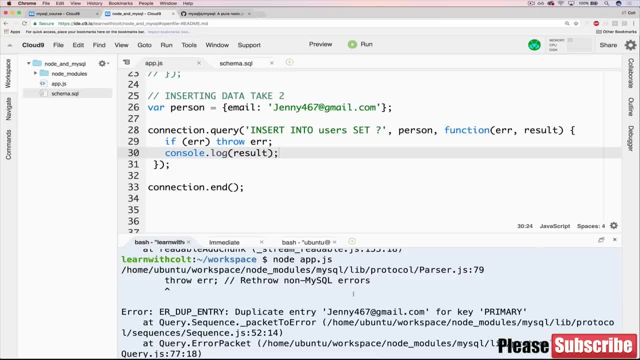 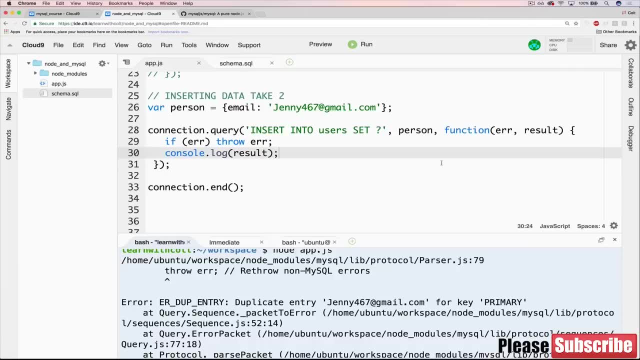 And this time it came back saying there's a problem, And if we look at the error that it threw, it says duplicate entry for key primary. So you can see now how JavaScript is talking. This is the kind of remember those arrows. I won't go back to the slides, the two way arrows, where 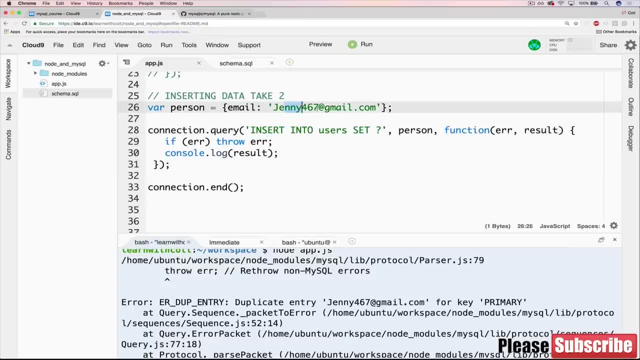 we tentatively tried to insert from node- hey, can we insert Jenny 467?? Waited until it went to the database. The database said: let me think: No, sorry, We already have Jenny 467 and there's a primary key constraint. 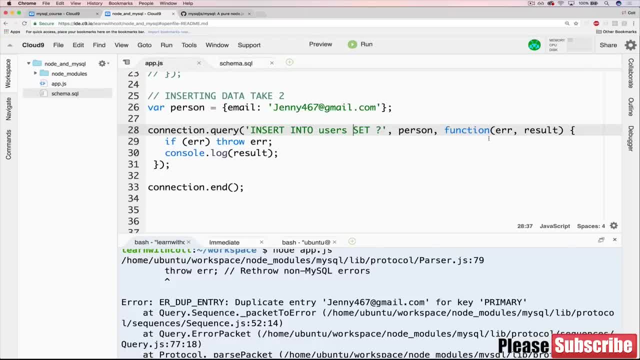 Don't you remember? you made the schema. Well, that's a problem. I'm going to have to refuse your request and send you back an error, which then is passed into this And this part runs. if error, throw the error. 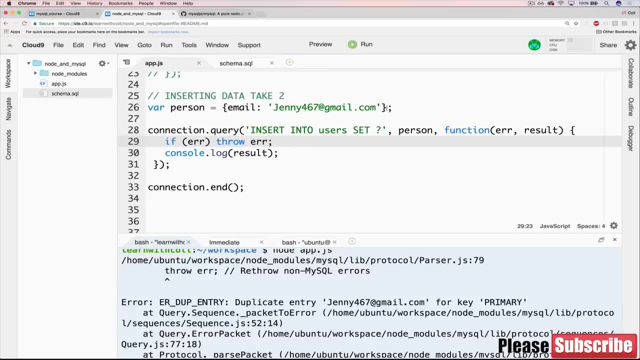 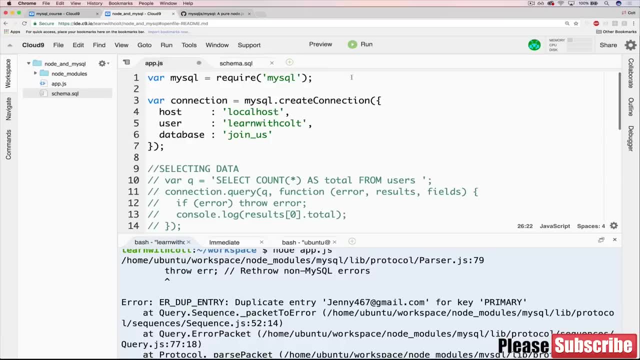 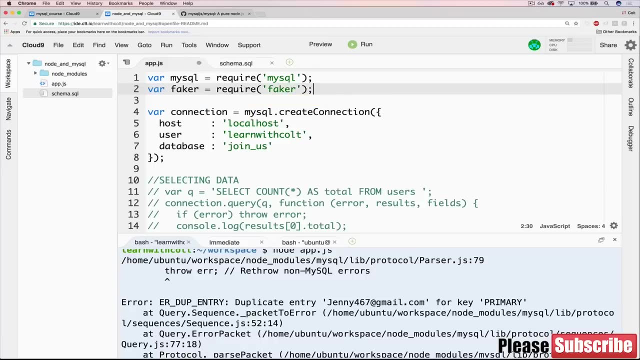 Okay, cool. So that's good to know. it's working. So, rather than doing Jenny 467, let's change this to something more interesting. Anyways, let's go back to using Faker. So we need to require Faker again, require Faker. 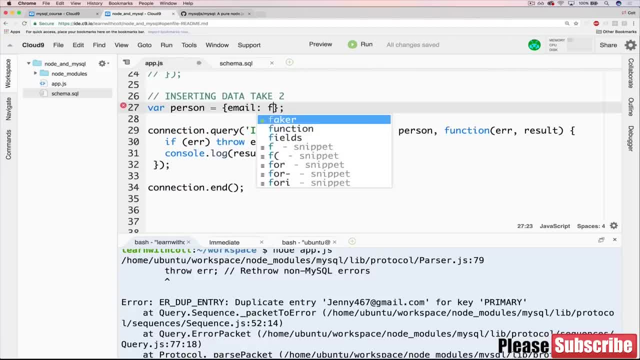 And all we'll do is insert someone with a new email. So it's just Faker dot Internet dot email, like that. So what this will do Is, instead of having us hard coded, every time we run this file, it will insert a new email that it just generates. 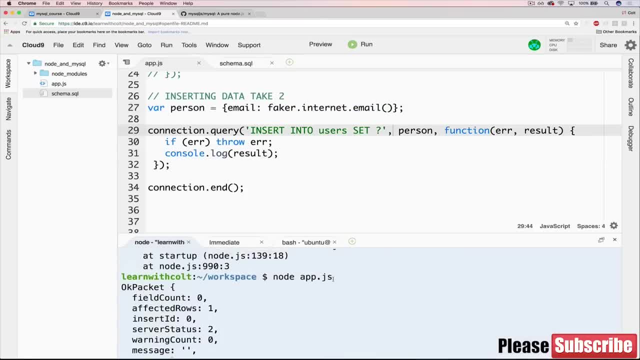 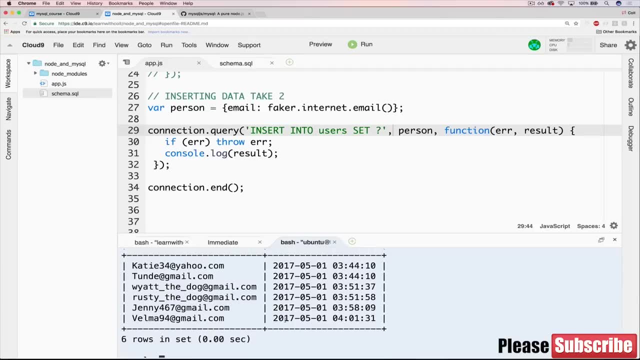 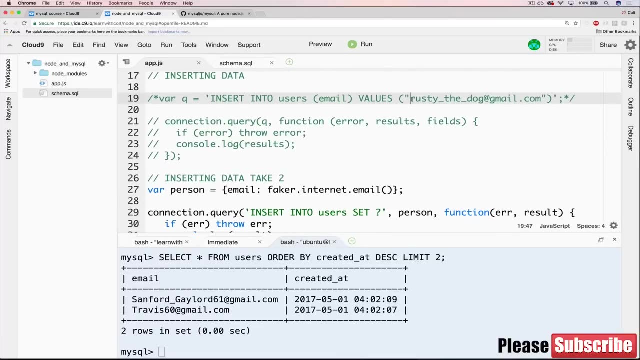 So let's try it see what happens. Okay, it looks good. Something happened. Now you can see we got Velma 94 at Gmail dot com, And let's do. how would we only identify the last one that was most recently added? quick review: 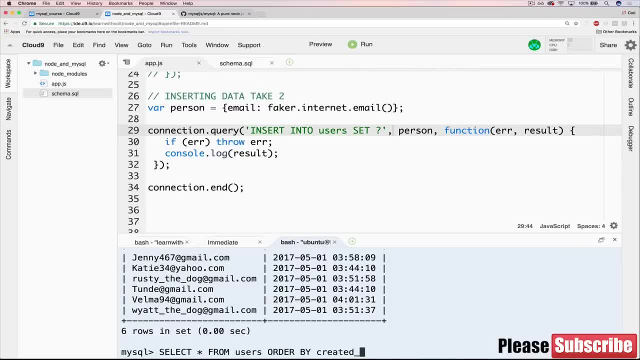 Well, we could. We could do an order by created at. if we did it that way, you can see. the last one is Velma. We're going the wrong order. so we can do descending And we could throw in limit one. Now we get the most recent one. 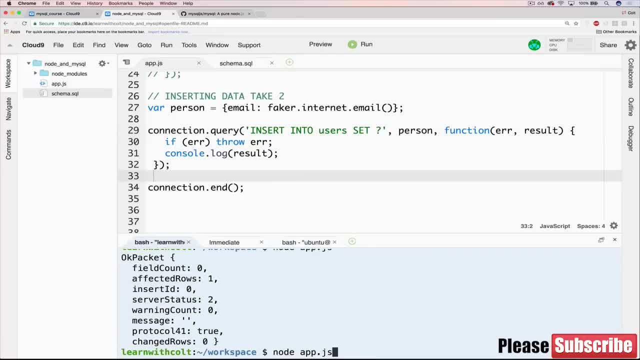 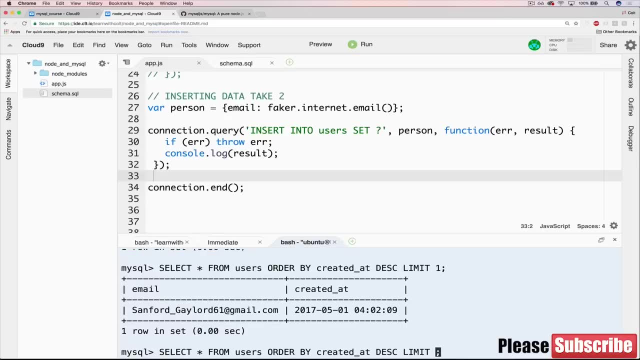 So if we go back to bash, try running it again and again. We've got Sanford Gaylord 61. And actually, if I change limit to two because we just inserted two, we also have Travis 60 at Gmail Dot com. 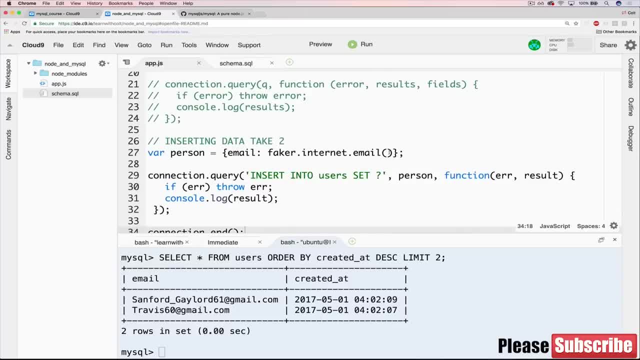 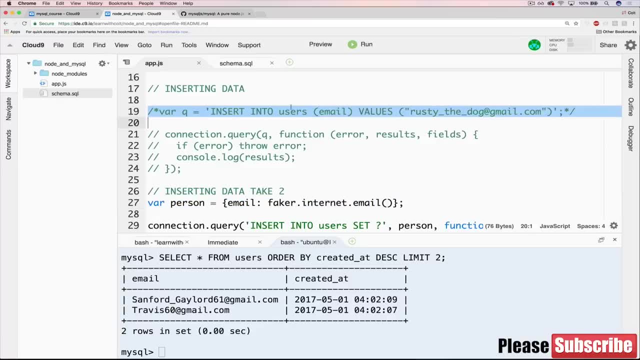 Sweet. So I'll end the video here. But we saw now how we can insert things dynamically and why this syntax is preferable, preferable to this one up here, where we're hard coding it as a string, as text. This works, but it's limited, right. 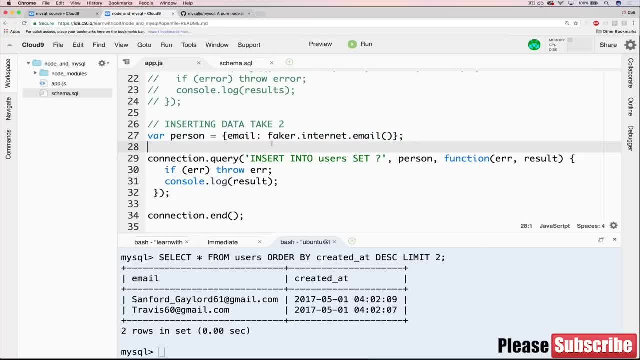 We can only insert whatever we type. This allows us to be dynamic And shortly in our web application. we won't have faker dot Internet dot email. We'll have. this is pseudocode, whatever The user entered into the form. So when we have that form the user enters their email. 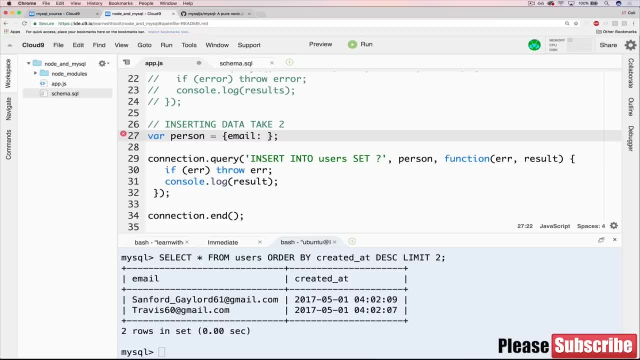 Whatever they type in there, we're going to stick here. and we don't know it, Right, We can't type it out exactly, We don't know what the email is itself, but we can save it in a variable. OK, so we'll go back to faker dot Internet dot email and we'll leave it there for now. 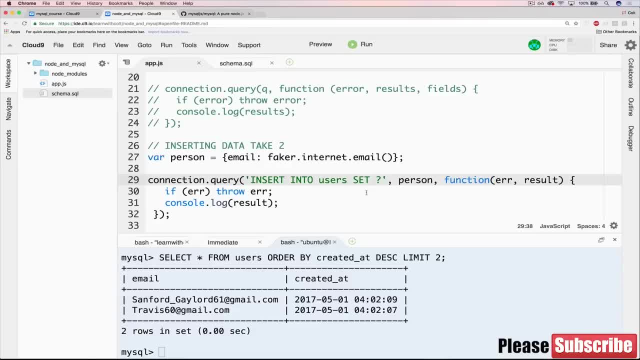 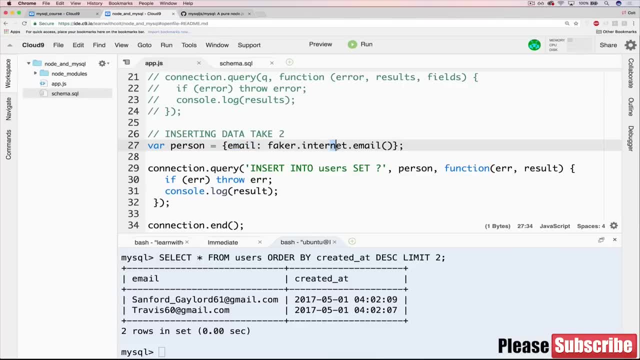 OK, so let's refresh what our master plan was here. The whole point of using faker was: eventually, we want to be able to insert five hundred of these Where we have an email that's randomized, and we also want to have a date created at date that is randomized. So let's focus on that part. 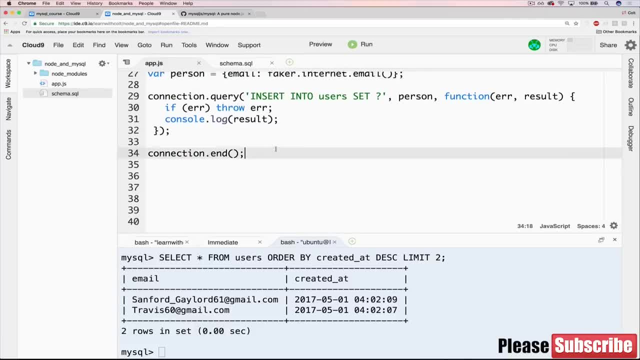 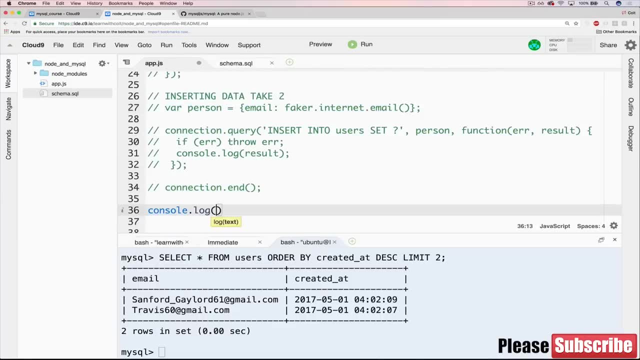 We saw, just to refresh your memory, that we can do things like this, Let me- I'm going to comment all of this out and to just run one line at the bottom, which is console dot log faker dot date dot past, And that just gives us a date in the past. 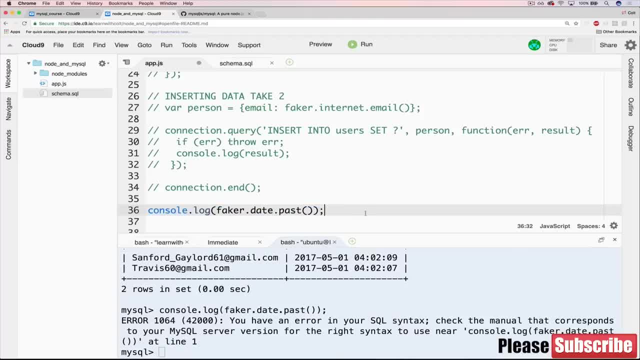 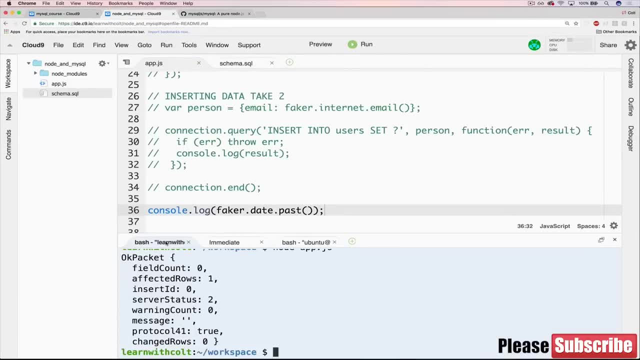 I think it's within a year and maybe two. And let's see what I'm screwing up here. Got faker dot date dot past console dot log And we'll go over to the correct terminal here and we'll run node app dot JS. 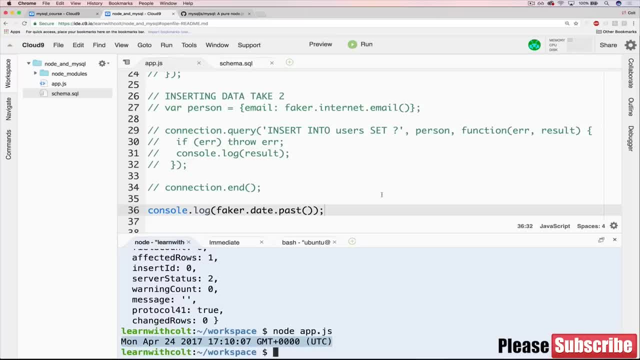 OK, now we're getting a date. Now you may have noticed a problem here, This date syntax, which I'll put here just so we can take a look. It's not valid JavaScript as it is. It's complaining, but this is not going to jive well with our database. 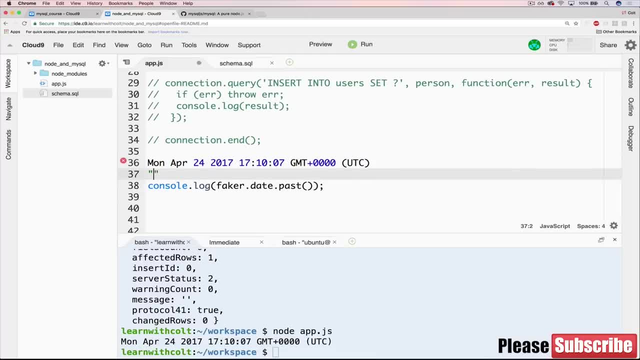 Remember that our database, my SQL, is expecting something like this: where we have the year, I'll just do it as year: year, year dash, month, month, dash day, day, space, minute, or what do we have? our hour, minute, minute, second second, So sort of in the time part looks OK. then we got all this stuff that we don't want. 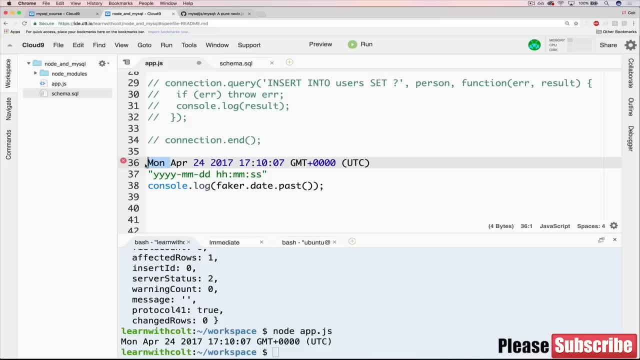 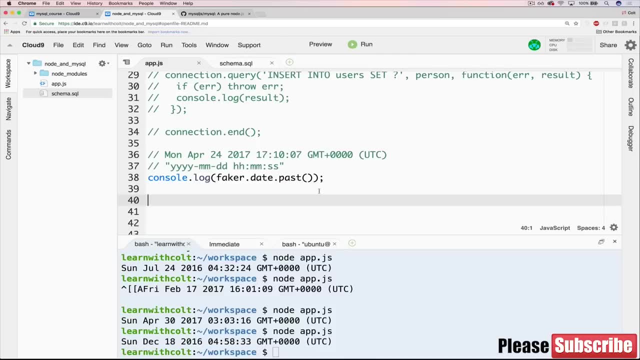 the year, though the month, The day of the week. we don't want the month spelled out, we just want the day. So this is a problem. So, to prove that it's problematic, let's try something. Let's try taking, say, this date right here. 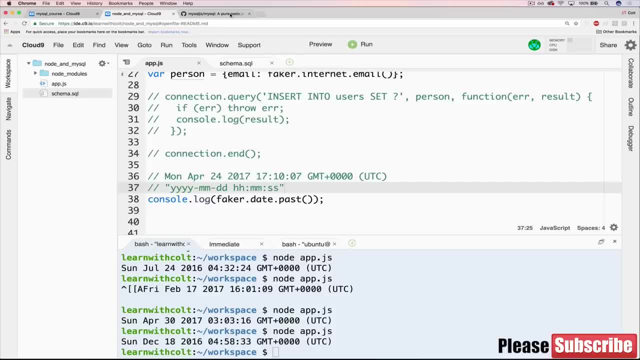 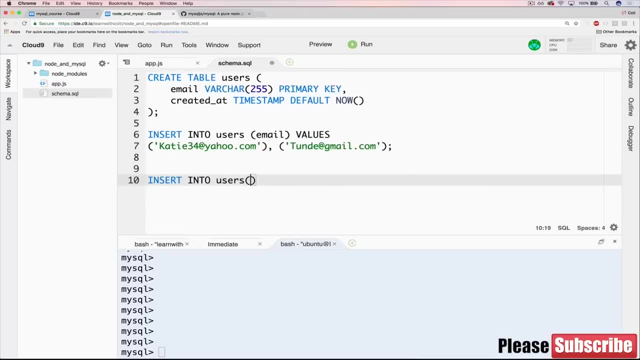 Monday April 24th twenty seventeen. Copy it over and let's insert it manually into my SQL and see what happens. So I'll do an insert into users. We have email and created at Values and we'll just pick a random email. 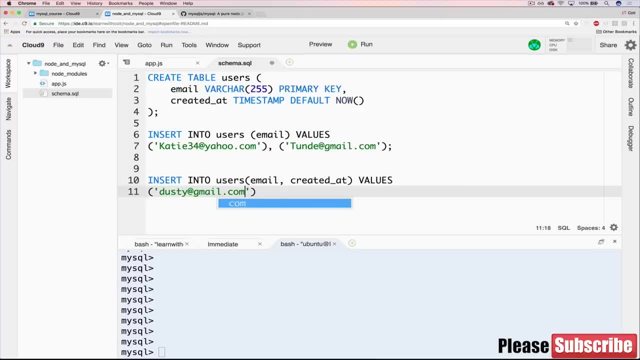 Let's do dusty at Gmail dot com comma, and then we'll pass in this giant JavaScript date or the JavaScript style date string. What do you think will happen when we insert this? So I'm just going to paste it in And hit enter. All right. 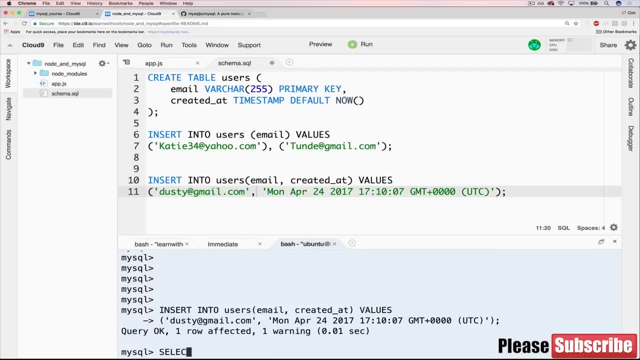 One row affected one warning. Well, let's see what happened. Let's do a select star from users. Actually, let's do select star from users where email equals Dusty. at Gmail dot com, And look at that created at is all screwed up and sent it to zero, zero, zero, zero zero. 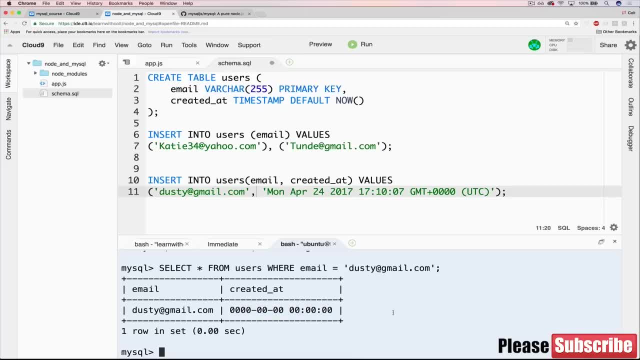 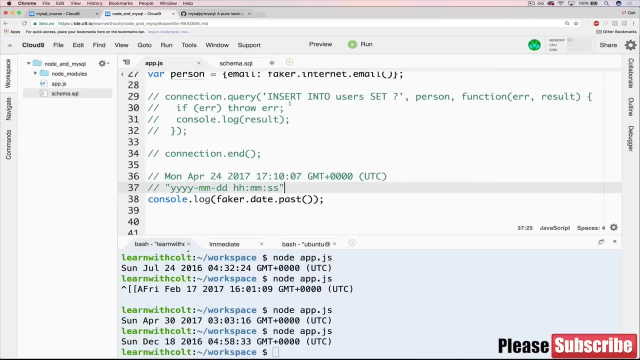 It's a problem That's not going to work for us. It's wrong, Right. So that's proving to you. our point of this is to show you that the JavaScript way of doing dates that we get from Faker is not compatible with my SQL. 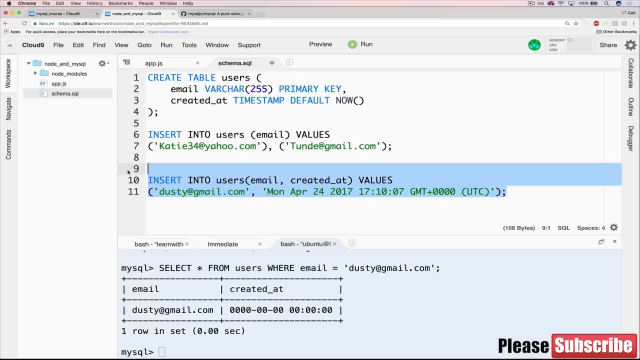 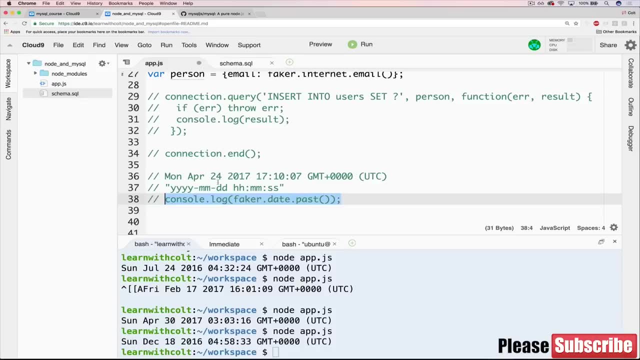 So let's just see what happens. I guess I can keep this here. Let's see what happens If we go to our app JS and we try and insert A person with a faker date. What do we get? an error message or what happens. 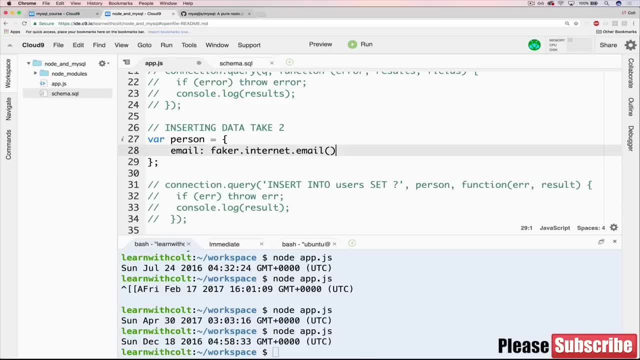 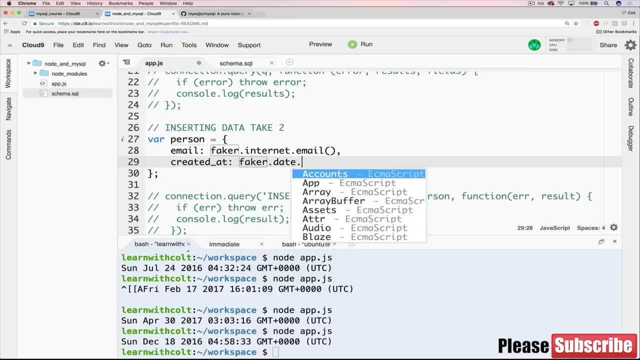 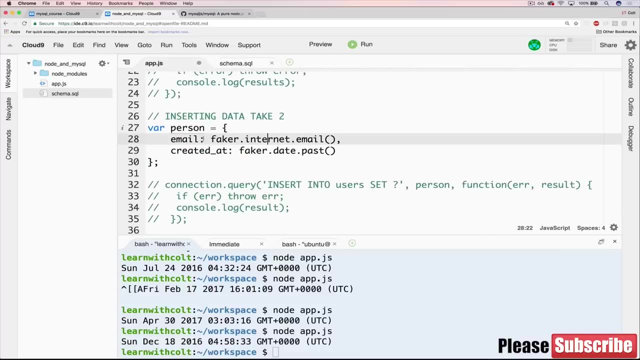 So we'll do this, make some space here, And rather than just email, we'll also do created at Which is faker dot date dot past. So the same thing we did down here which generated this date, But now we're doing it dynamically here with an email. 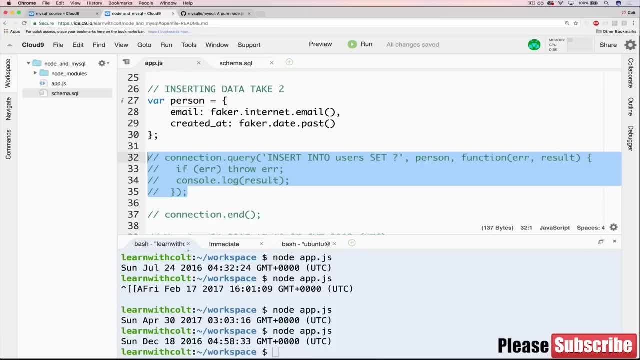 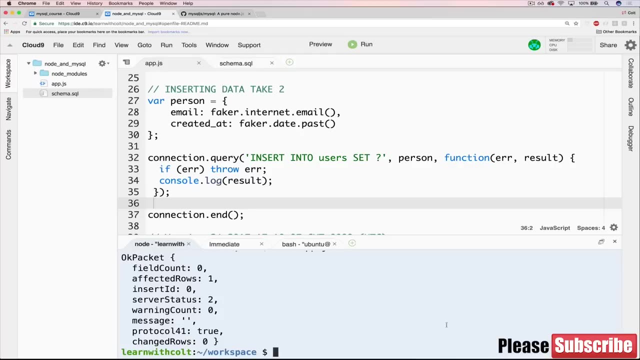 And a created at date, both dynamic. We're going to insert person using the same syntax And let's see what happens. Okay, Hold our breath here. Node app JS And what do you know? We don't get an error. So what's going on? 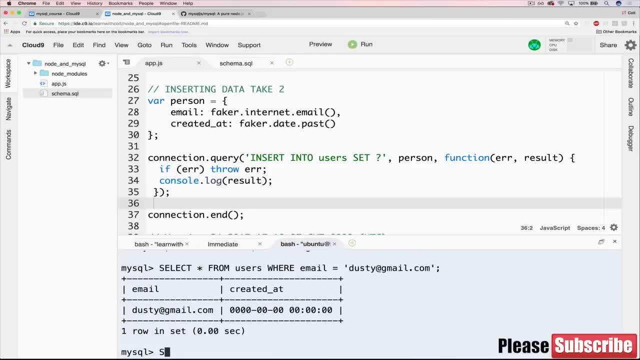 Did it work? Let's come over here. Unfortunately, we're not able to do our select star in order by created at, Because our created at dates now vary, so it's no longer that the last one added in has the most recent date. 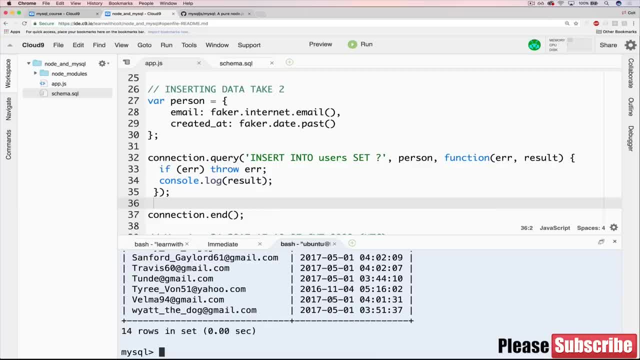 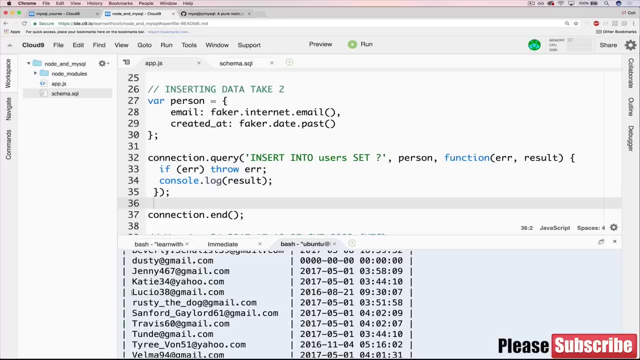 So we'll just do a select star from users And what we'll look for. in my case, I happen to know the data that we're working with. This was the one that was just added, Lucio 38,. yours, of course, will be different. 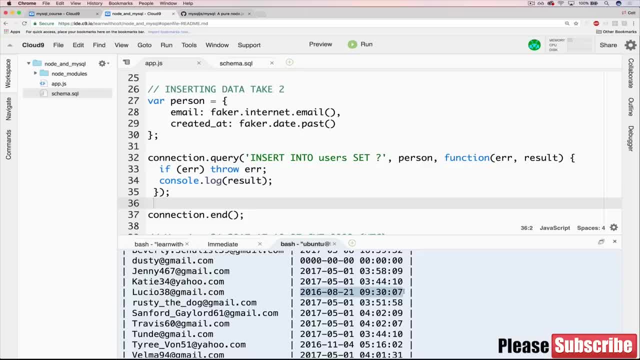 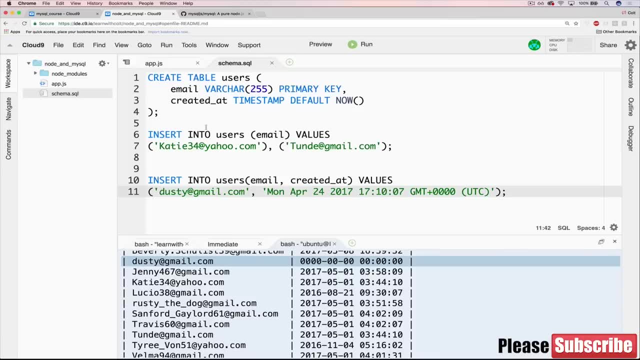 But notice that the date time of the created at isn't zero, zero, zero, zero, Like we had for Dusty. This is the one where we manually took this. the same exact thing coming from JavaScript, But we did it ourselves and didn't work. 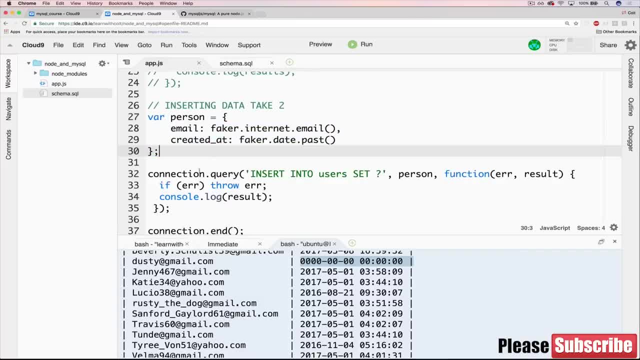 But then when we used person instead of variable, then we use connection query and we passed it in, it somehow worked and basically it comes down to the magic of this library, And I'm showing this to you to illustrate another point, which is there's a lot of 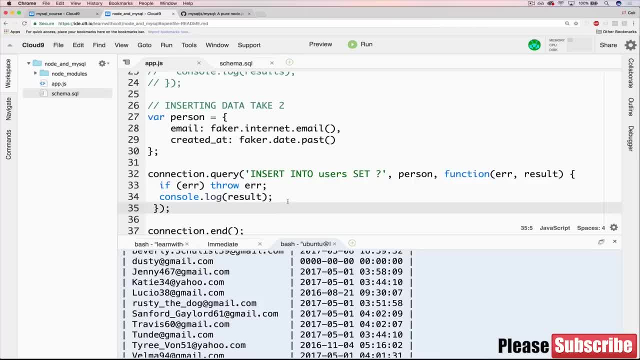 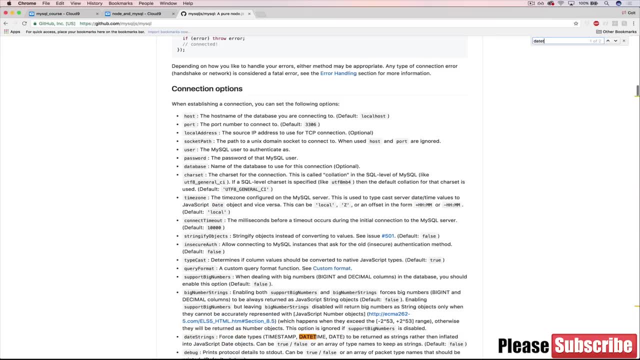 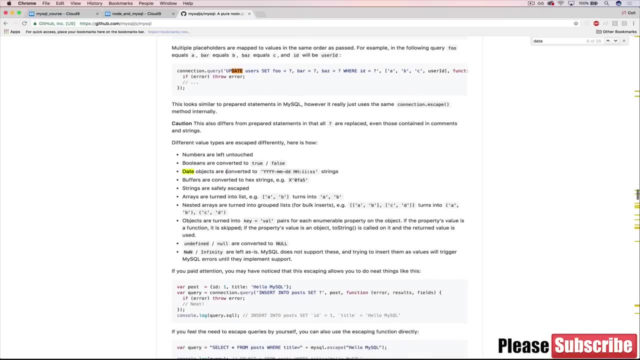 work that goes into sewing the stitches between something like node and MySQL. So if we go to the docs here, if we do a search, for I'll just do date time And I think it's down. OK, here we go. If we look, there's something right here that says date objects are converted to. 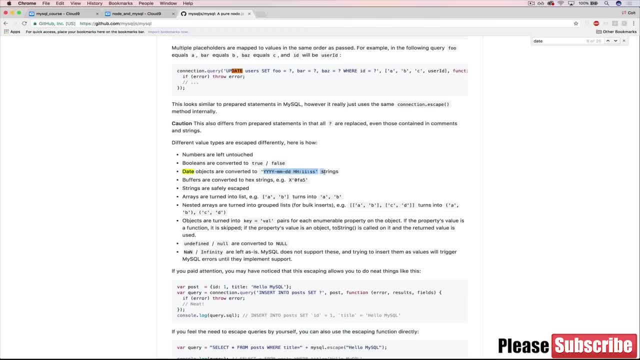 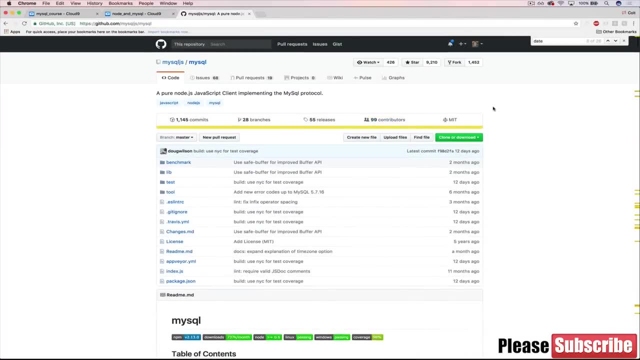 year, year. year year dash month, month, dash day date- Basically the syntax we're looking for. they're converted to that. So, as part of this library, it takes it upon itself to bridge MySQL and node It's. it says: all right, if this is a JavaScript date, which is what we're. 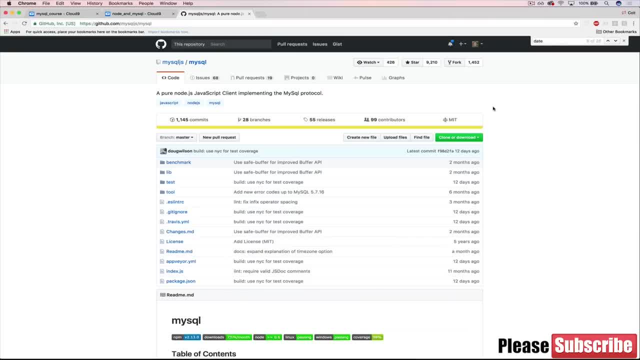 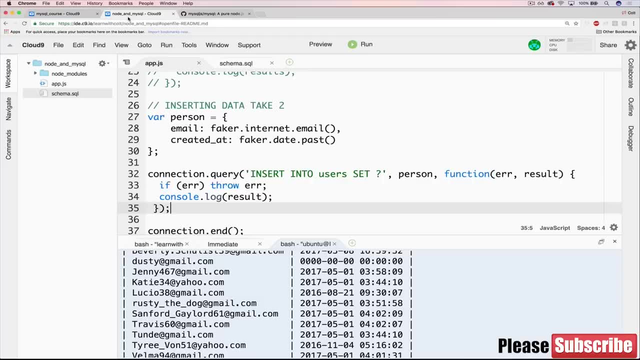 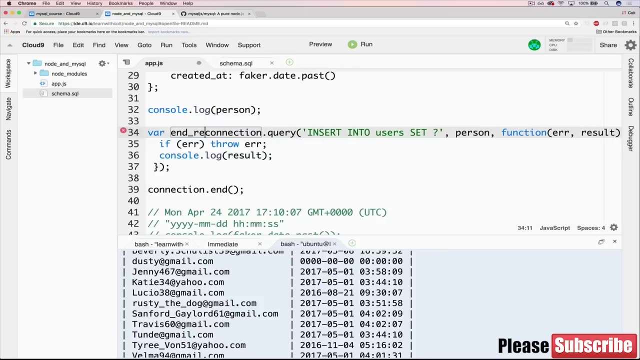 working with from Faker. well, I know that the user is trying to insert it into a MySQL table that has no idea about JavaScript dates, So we're going to convert it before we send it. And then one other kind of interesting thing we can do is save this to a variable and we'll call it end results. 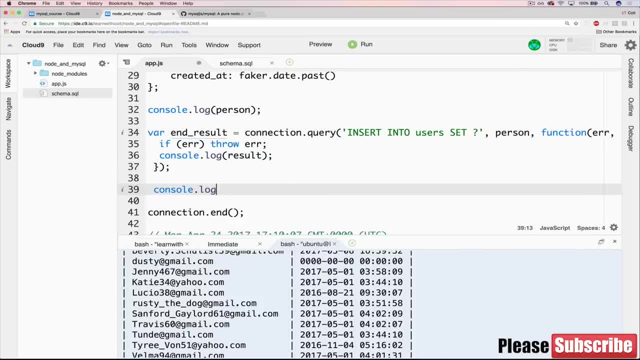 And if I just do a console dot log And Result dot SQL- which again all new stuff, I know it can be overwhelming. What this will do is show us the compiled sequel that is being sent over, And so this is kind of before what person looks like. 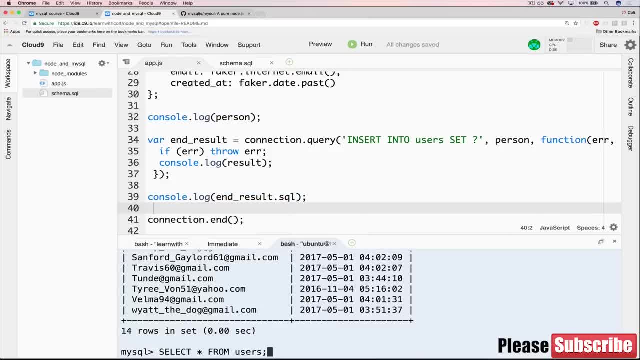 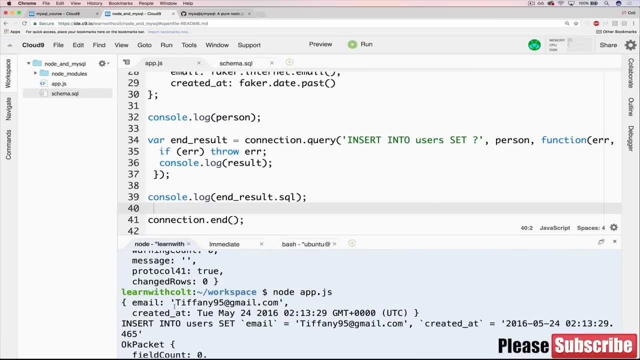 And this will be an after. Let's take a look. Well, we have to go to node. OK, so you can see. before we had created at looks like this, Tuesday May. it's the wrong format. that's JavaScript format. 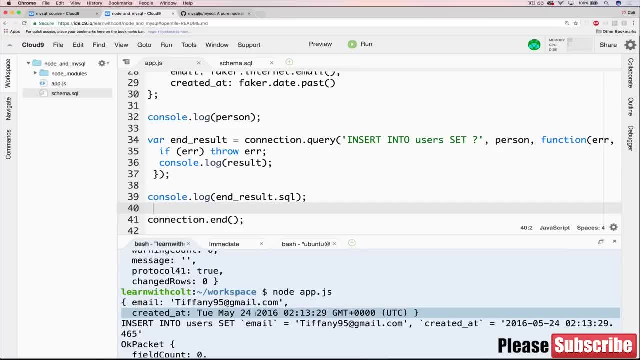 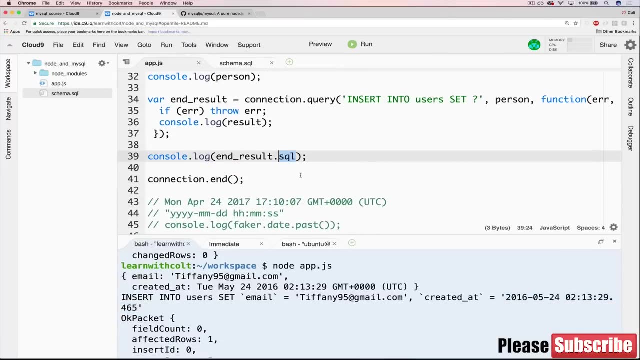 But sometime before we actually sent this over, it was converted to: created at is equal to twenty sixteen dash. oh, five dash twenty four, And this is the correct MySQL syntax. So this is kind of cool to be able to see the end result: sequel that's being sent over. 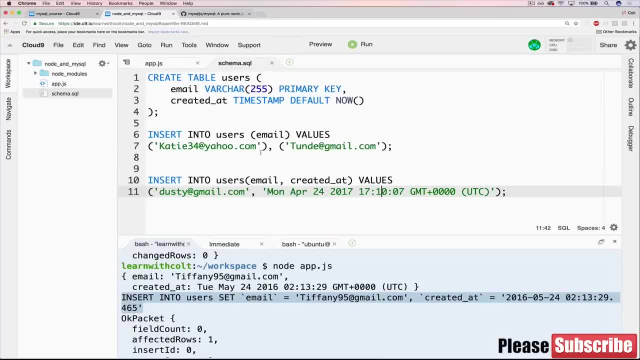 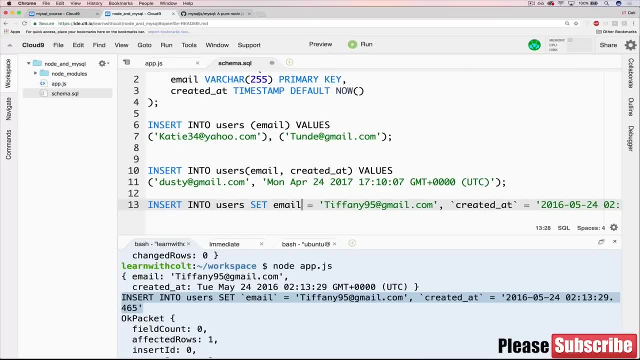 This is a valid sequel that we could just copy this over And, yeah, it might look slightly different. These are escaped, which you do not have to do, But if you notice, this is a sequel syntax and we could just paste that in. 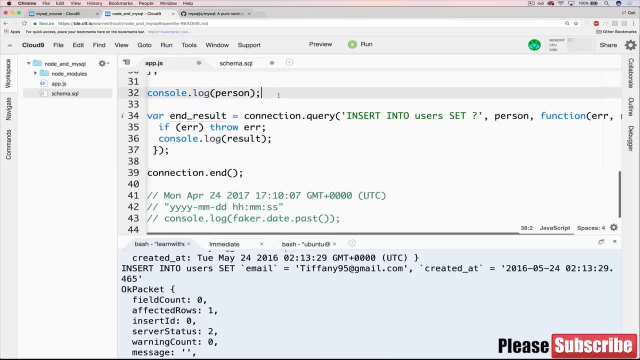 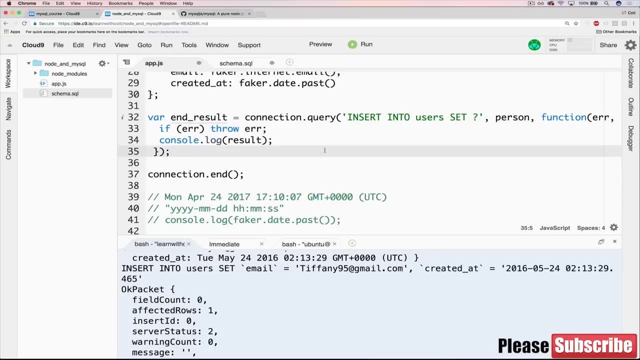 OK, so I'm going to get rid of that, But I just want you to see that you could do that. And, more importantly, the whole point here was to show you that there's stuff happening behind the scenes which can be great and useful, but it's also there's stuff that you just 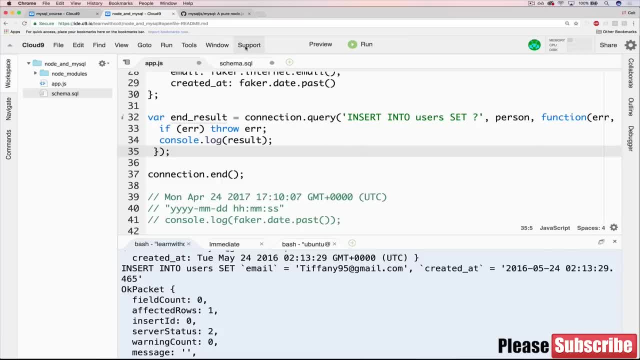 don't know what's happening sometimes and you run into it, you discover it. But it's the job of these libraries to connect the two And there's a discrepancy in this case between how JavaScript handle states and how MySQL handles or expects them. 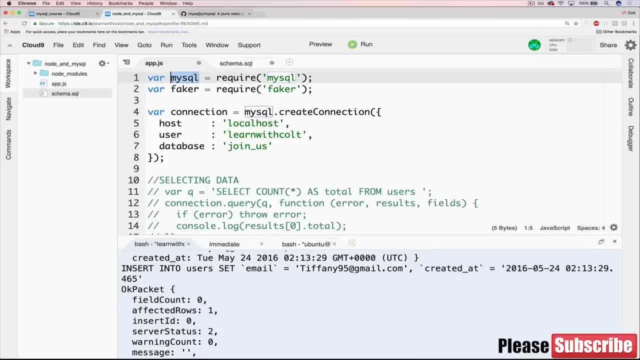 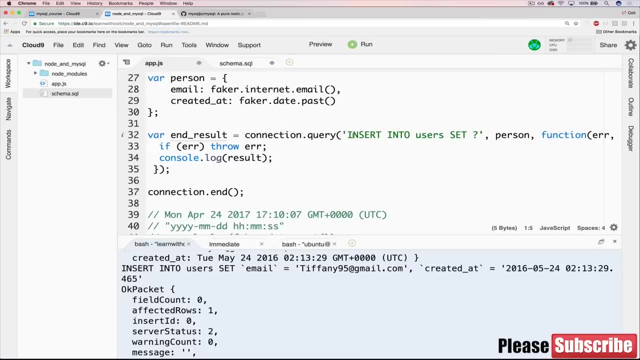 So, behind the scenes, this library that we're not writing, we're not in charge of somebody, is that library is patching them. It's fixing it for us. OK, So we've inserted a single user. Now all we have left is to figure out how we insert 500.. 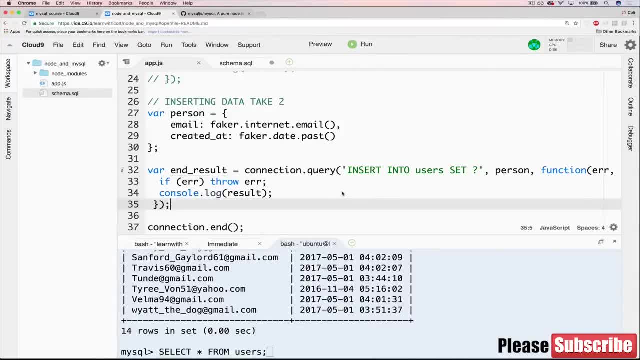 That's the next video. All right, So we're finally at the end of the section where we're actually going to insert 500 users at once, And you'd think that it'd be easy, because we already saw how to insert a single user like this. create a single object. 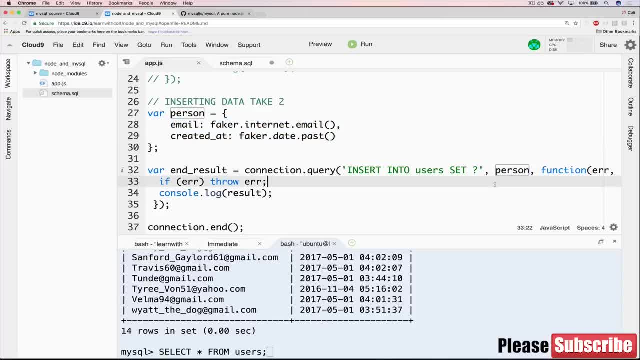 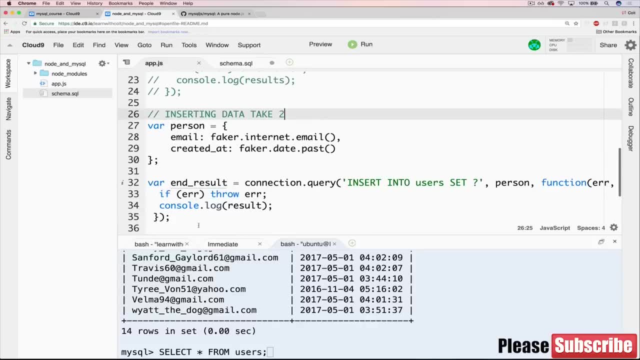 pass in email and created that and we just pass in that single one. But then we have to worry about OK, well, for trying to do 500, technically, what we need to do is repeat this entire process 500 times. But there's a better way than that. 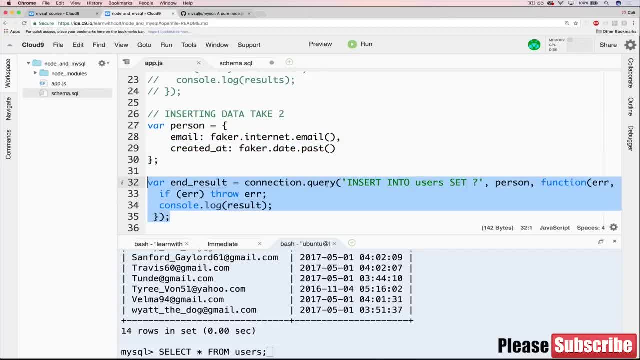 because, if you think about this, every time we're running a query here, that's 500 separate queries, inserting one at a time individually, which is not ideal. What would be much better is to generate all 500 users at once and then do a bulk insert. you know, insert them all together, like you know, like this: 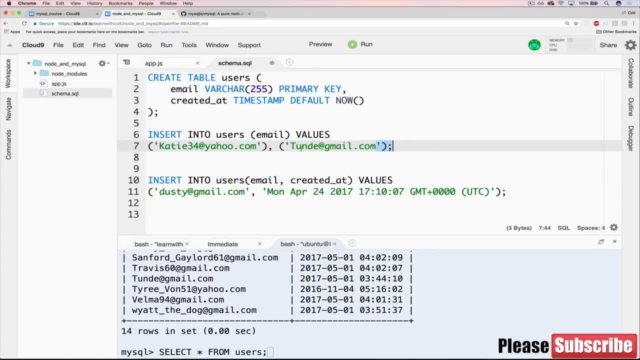 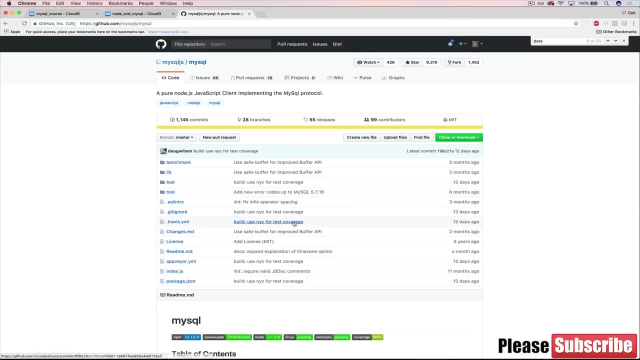 Here we inserted two, not 500, but this is two people being inserted. We're passing in a list. Now. this is MySQL, though Now the way we do that in Node using this library, is a bit different, So I'm going to show you. I dug through. 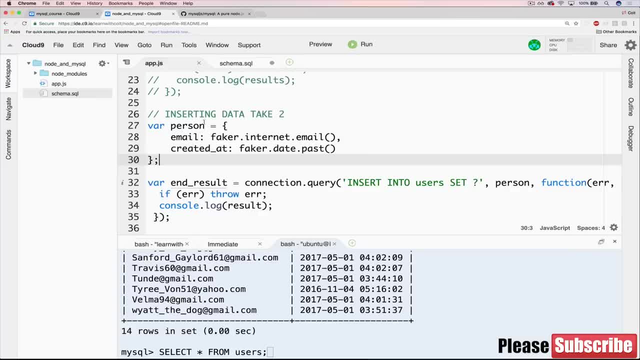 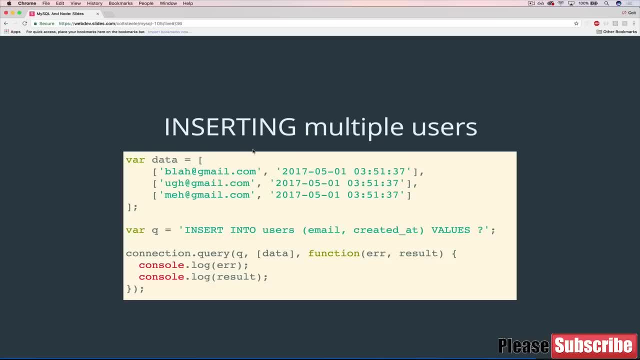 the documentation and found out how to do a bulk insert rather than passing in a single object like this. but it's actually expecting is an array of arrays, So something like this here. So I'll show you a better example. We'll actually do it together. 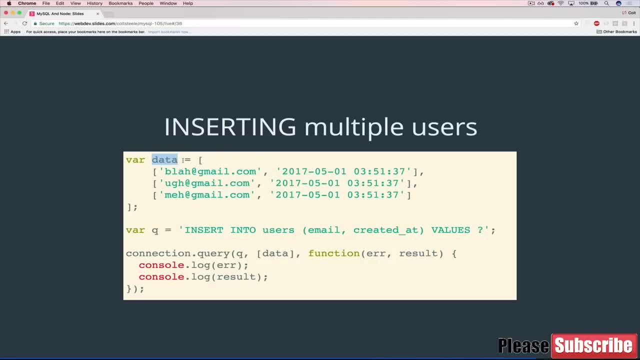 But rather than giving it an object, here is an array called data. Inside of it, three separate arrays. The first thing is an email, The second thing is created at. Then the query that we're doing is now insert into users, And we actually do have email comma created at our traditional syntax. 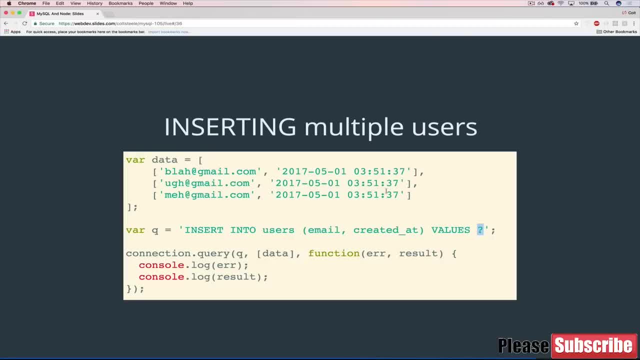 followed by values, and then this question mark will be replaced with whatever comes after it, which is data. So then we'll take this array here and it will stick it here and basically it will insert each one of these as its own row. 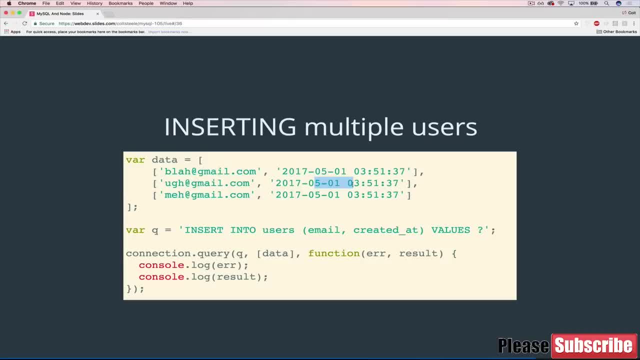 So we'll say: this is email, This is created at insert that. here's email created at insert that. So this is the JavaScript way of bridging that gap. This is how it's done with this library And this is why it gets wonky and weird when you're working with other libraries. 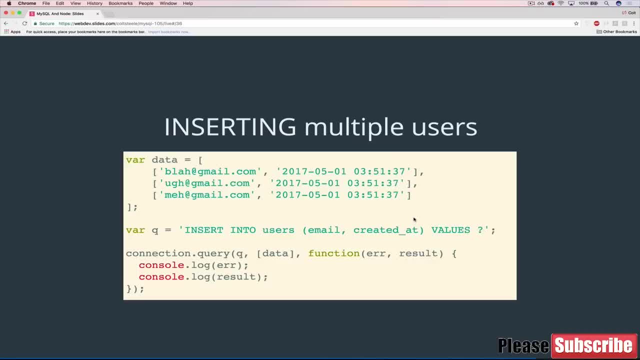 and other languages where they don't you know the syntax is different. They don't support the exact same way that you would work with my SQL. So it's kind of weird. But once you do it and you have it done, you can just refer back to the code you previously written. 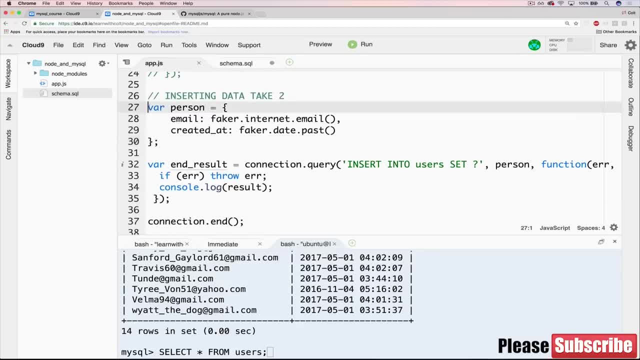 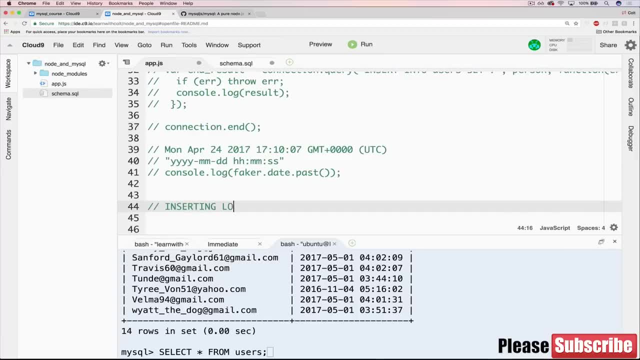 So let's test that, Let's see if it works first. OK, so we had inserting data. Take two in a comment, that out and move down to the bottom Inserting lots of data. Just make this a little easier to see the division. 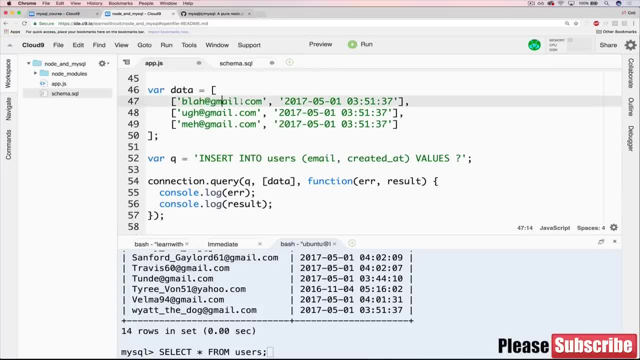 OK, so rather than just well, we can leave it as blog Gmail, I guess, and get Gmail and math at Gmail. So we have this array of arrays, only three. But the difference between three and five hundred is basically nothing. It's the difference between doing. 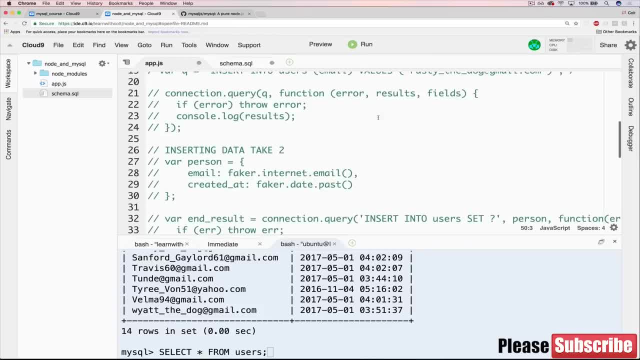 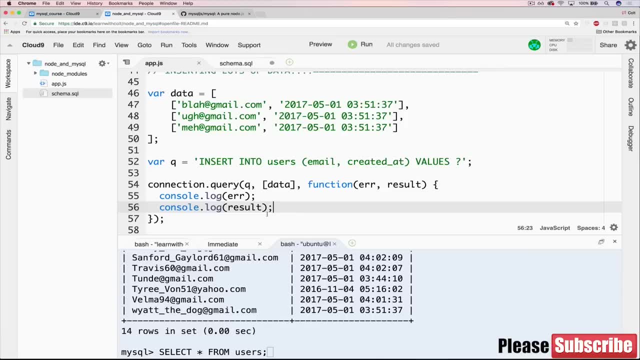 one and two that we're trying to get around right now. We saw how to do one, So this should be easy once we get three. So we save this here and let's just make sure that it works. I'll also add my connection dot end. 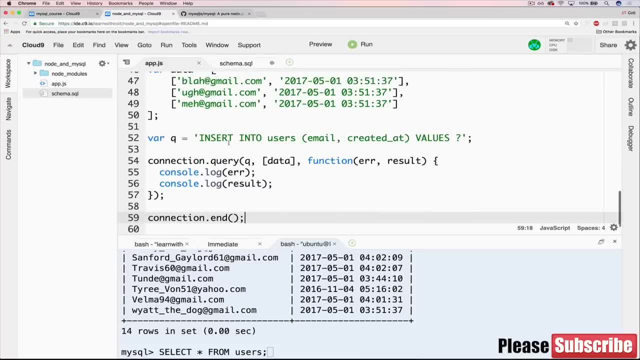 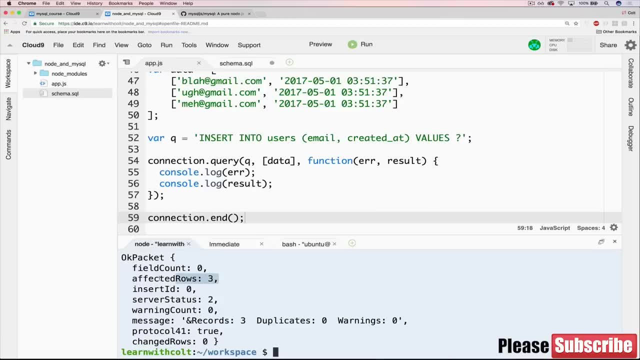 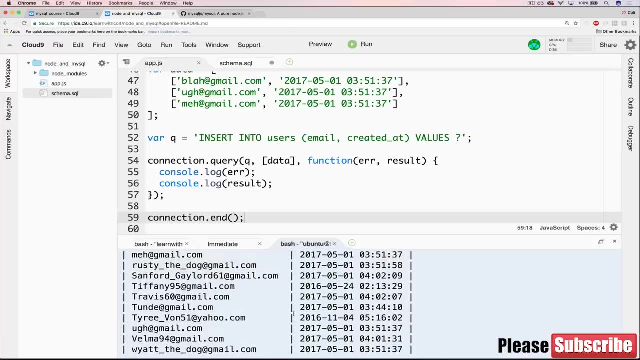 And we'll make sure everything else is counted out except the connection part and we'll run it from Our app over here. OK, it looks like three affected rows. that is good news. That means that they were inserted. If we go over here and do select star, 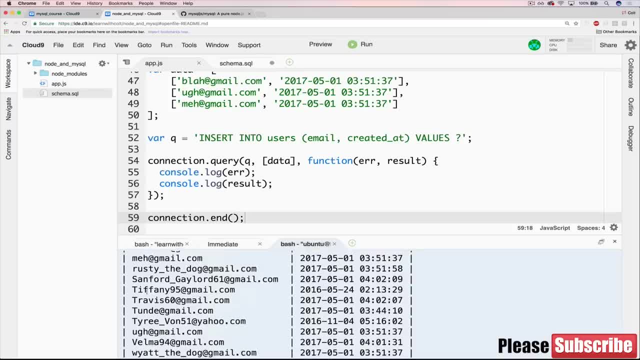 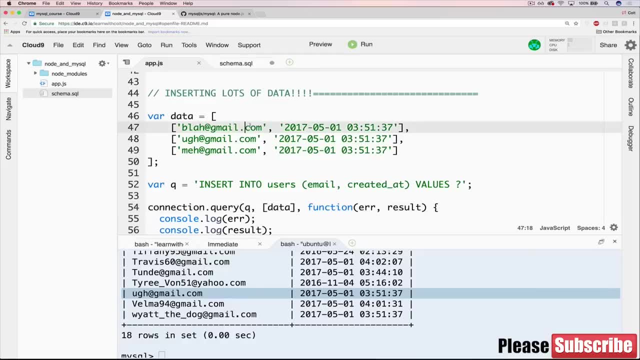 We can see math is in there and blah And where are you is at the bottom here too. So this worked. this successfully entered or inserted three. The syntax is weird. I totally agree. It's different. I totally get that, especially if you're new to JavaScript. 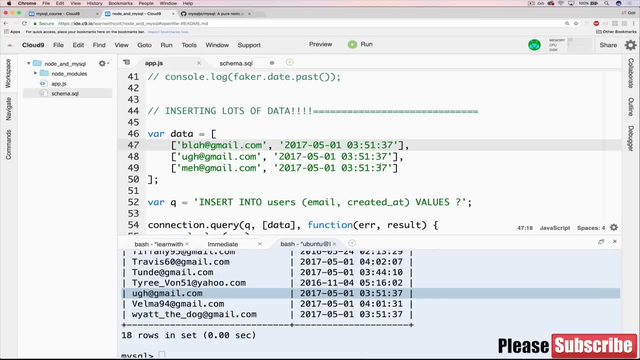 This must all be overwhelming. Don't worry, We're going to get through it. We're going to make the app. But what I want to show is that, again, it's different. You have to be prepared to kind of play within the rules of whatever language you're working in. 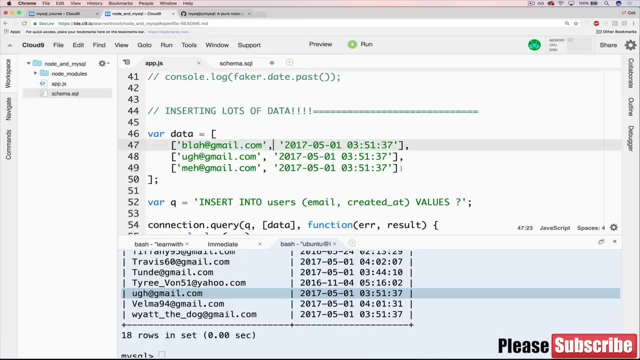 OK, so we've got this, but rather than these three, what we really want to do is generate an array with five hundred Entries. each one is going to have faker email and a faker date. So, to start, I'm actually going to make data empty. 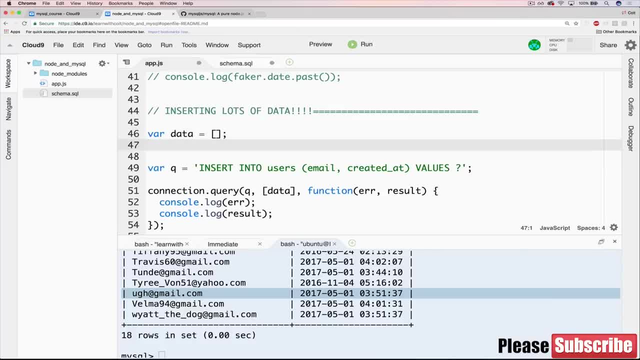 Just like that, And all we would need to do to add in our first fake array would be data dot, Push And push will just add to the end of this array. it will add inside of it whatever we tell it to. so we want a new array. 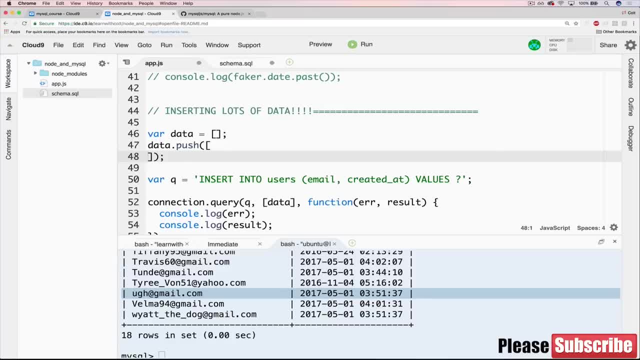 I'll make some space here, And all we want to do is push in two things. the first is faker dot Internet, dot email, and the second thing is faker dot date, dot past. So this will generate if we just do a single one. 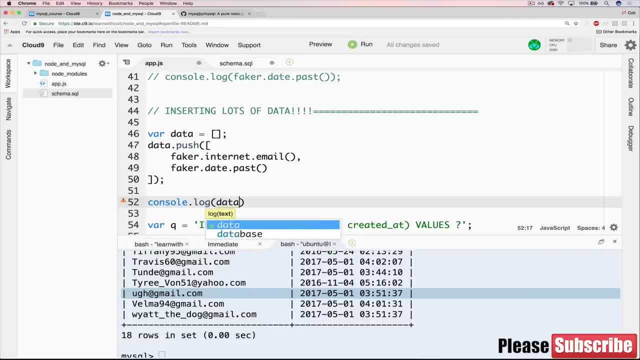 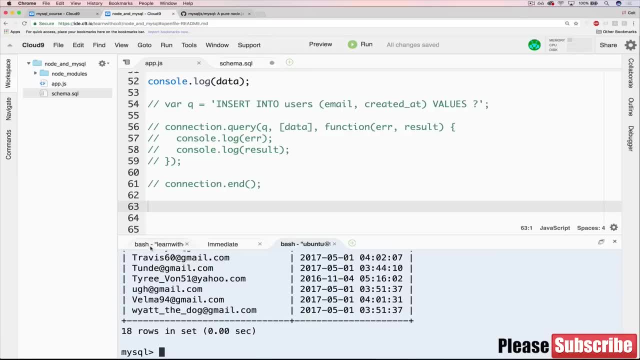 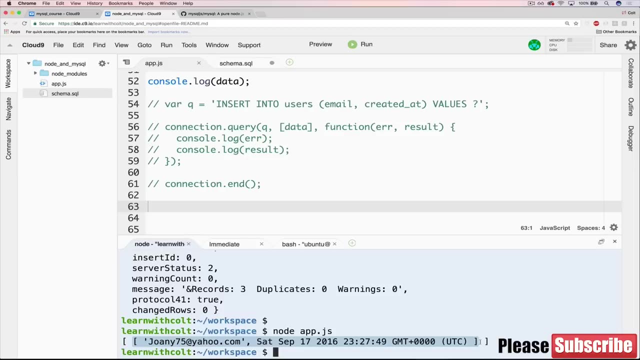 Oops, And do a console dot log data And don't do our query here. Comment that out. we run it wrong terminal. we run it, You can see. all right, it did it. We've got our first result in there. 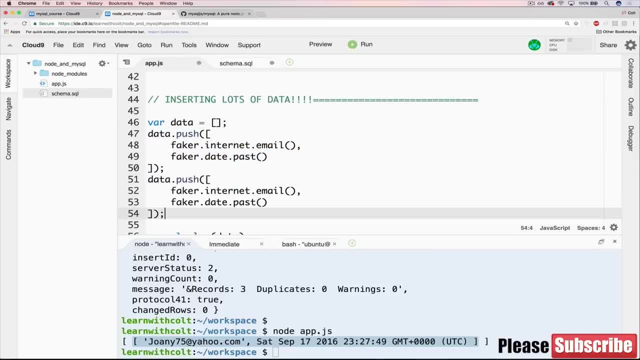 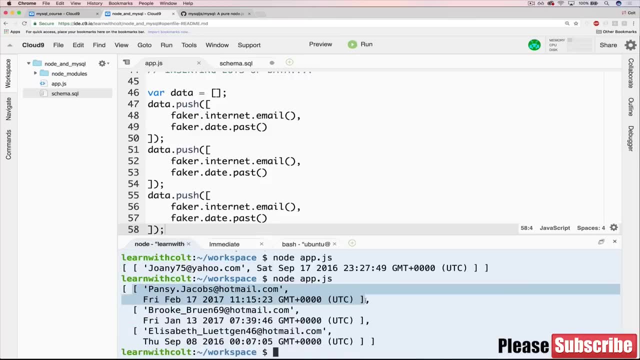 So then, logically, if we just repeated this and did another push, and another push, and I rerun it now, we end up with three. So we just need to do that five hundred times And we're not going to copy and paste five hundred times. 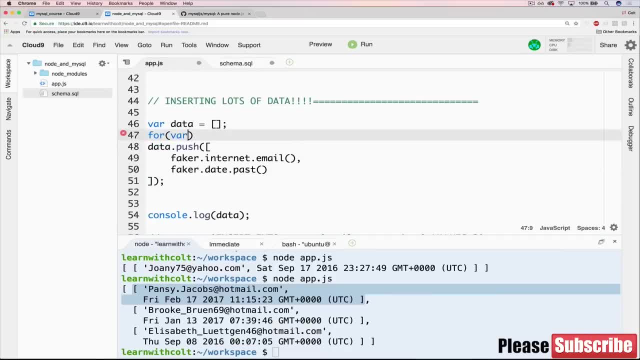 We're going to use a loop And it's just going to be a simple for loop. So for var, i is equal to zero, while i is less than five hundred. Add one to i. So we saw one of these earlier. If you're not familiar with JavaScript, these are the bread and butter. 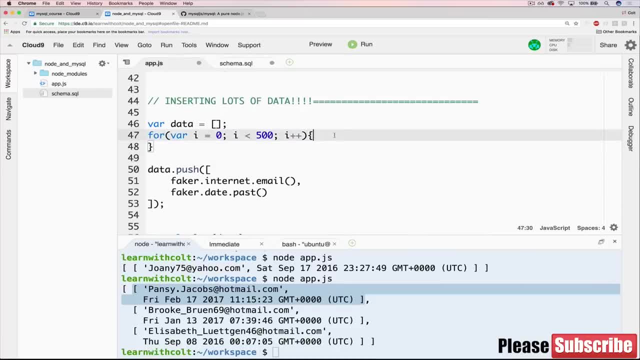 It's a way of repeating code. So this basically says: repeat whatever is inside of here five hundred times. So we just pass that in And this will now run five hundred times Each time it's going to generate a new email and a new date. 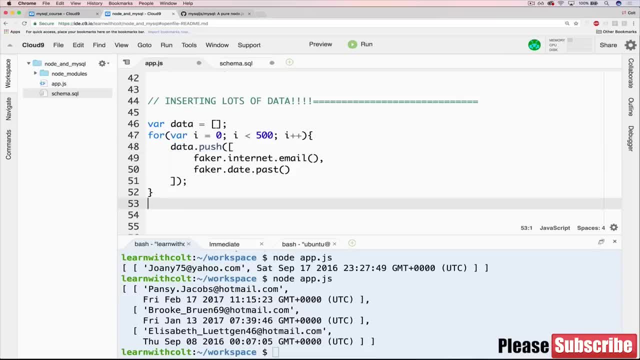 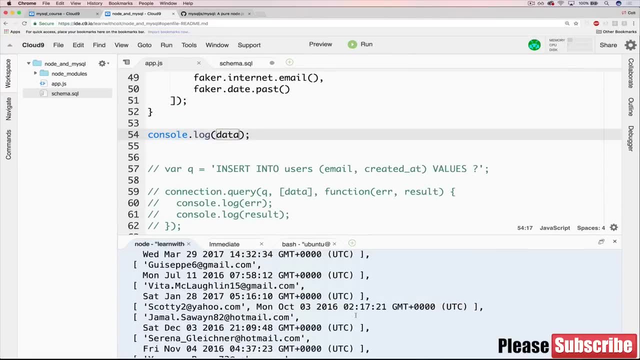 It's going to push them into the data array. So we end up with one giant data array so we can print that out. Let's see what happens And you can see as I scroll through here. you'll have to trust that. it's five. 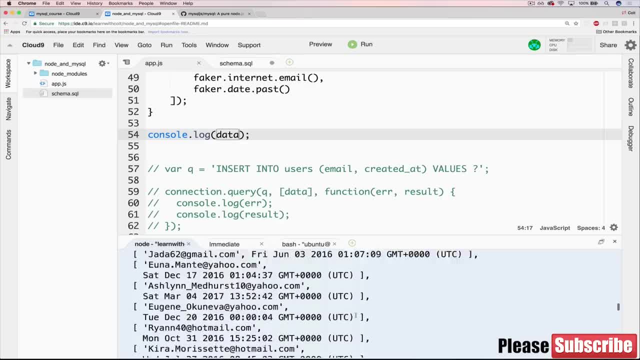 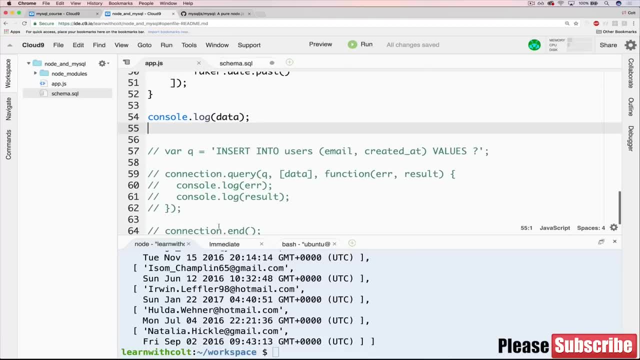 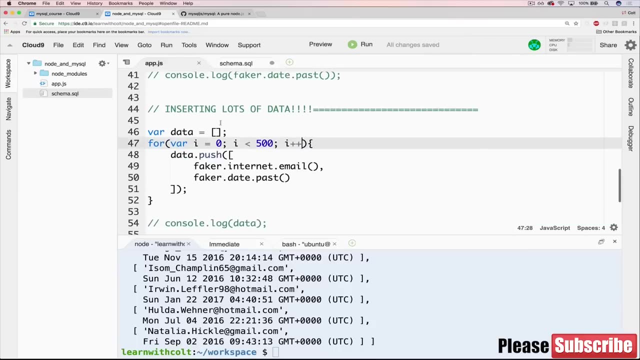 hundred. we've got tons of results in here, tons and tons of them- Awesome. OK, so now all we need to do is uncomment this section. I'm going to comment out dot log, but uncomment the part where we're actually taking that data. 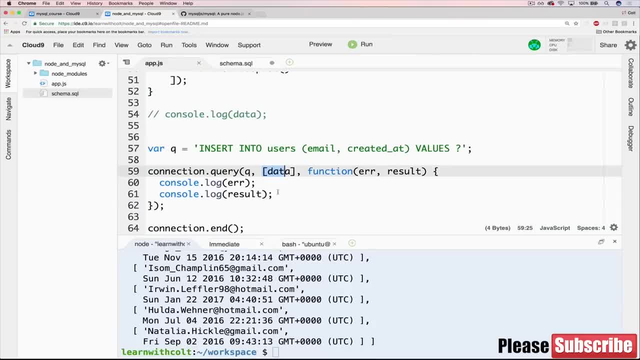 which is our giant array full of fake data, and we're inserting it And nothing needs to change. We have email first, followed by created, at right, If you look at our last one, email created. OK, moment of truth here. 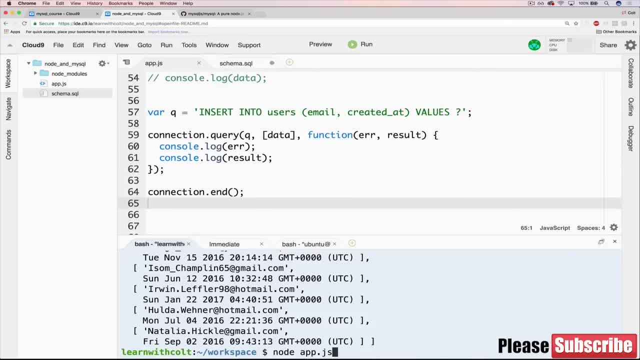 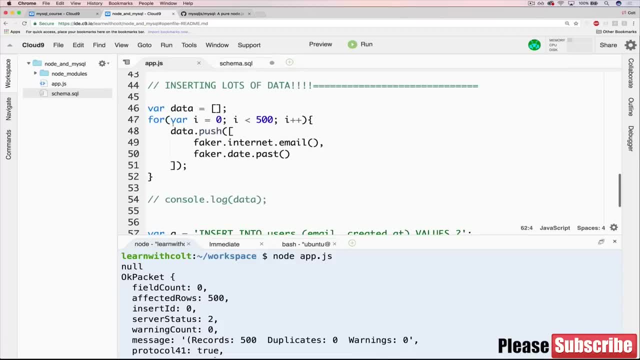 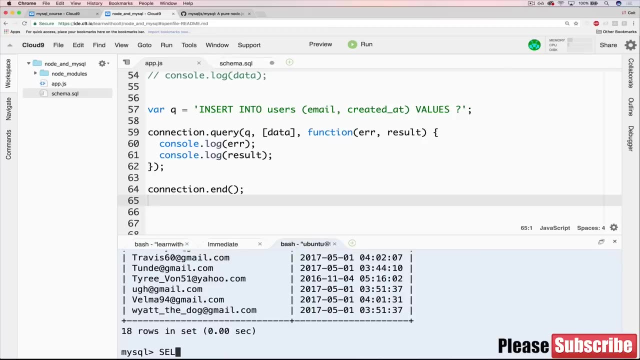 Let's try it. Save the file. It looks like five hundred effective rows. Look at how fast that was. Look at how short our code to do it It was. if you ignore all the white space, it's just this part. Now let's head over here. let's do well. let's start by selecting star. 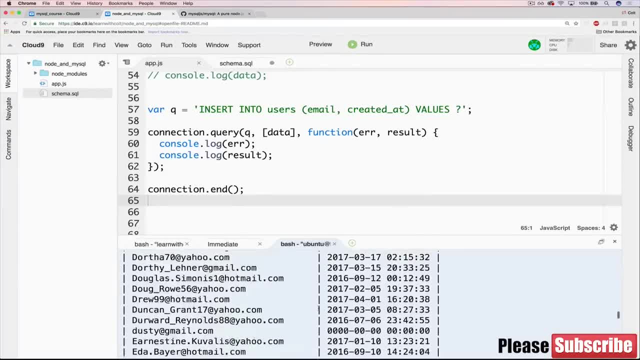 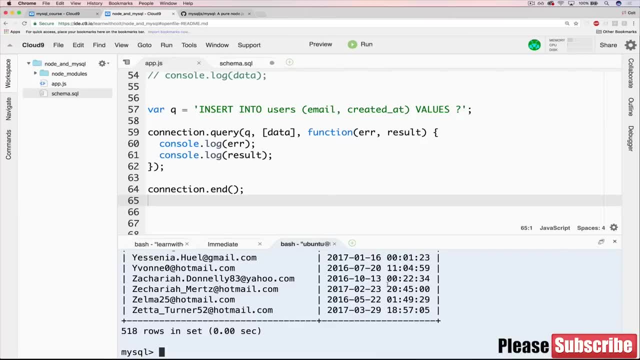 Awesome. Look at all of them there. And I'm actually going to drop everything because we have some bad users in there that, with you know, time created at set to zero zero, zero. so we're going to just do delete from users. 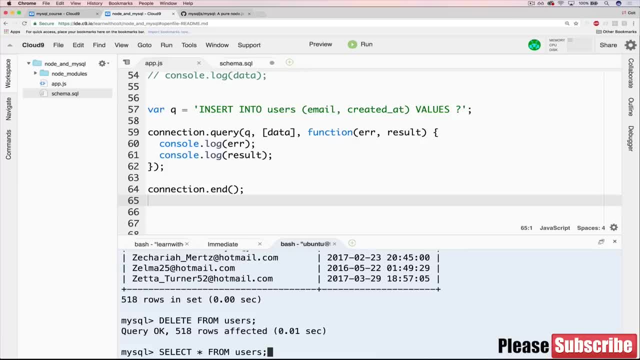 Five hundred and eighteen of them gone. now we do select star- Nothing, but don't worry, I'm just going to rerun our code one more time. And so easy, so fast. We now have five hundred users in there, Awesome. 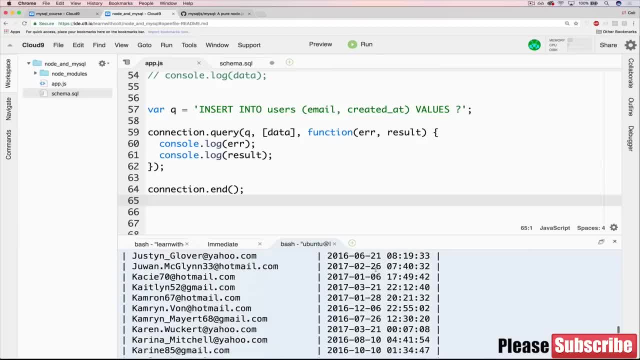 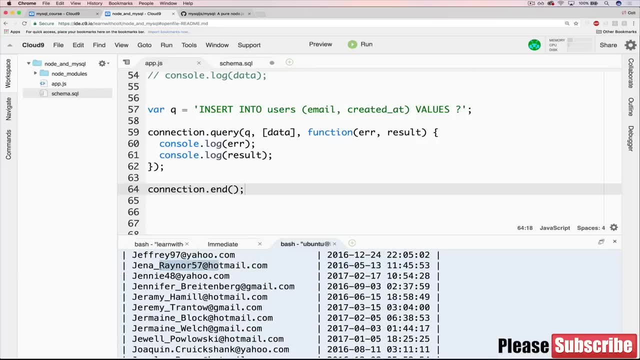 OK, so we'll end it here. I recommend that you delete everything and just remake it with five hundred Exactly. We have a couple of exercises using these. Of course, your data will vary, right? You're going to have different emails. 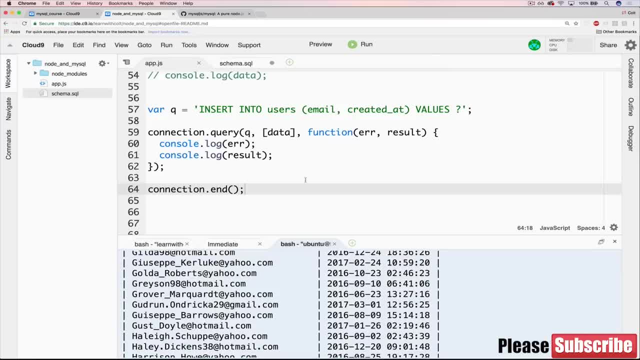 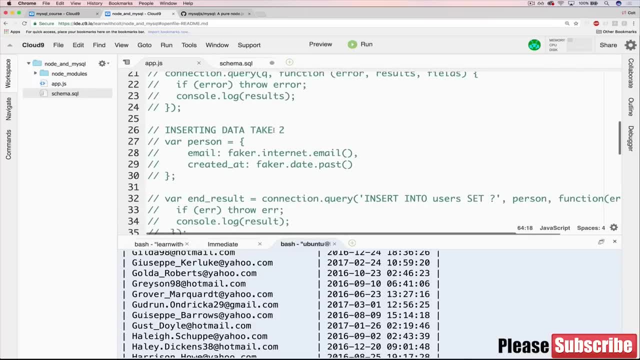 different dates, but it won't matter for the exercises And once we get past those exercises we'll move on to working with this data in the context of a Web application. So we saw a lot in this section. It's very kind of disparate, fast paced. 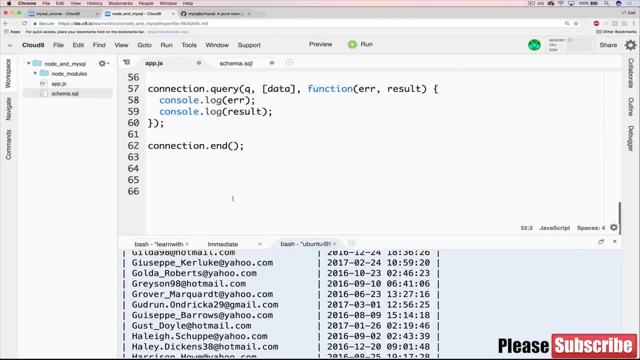 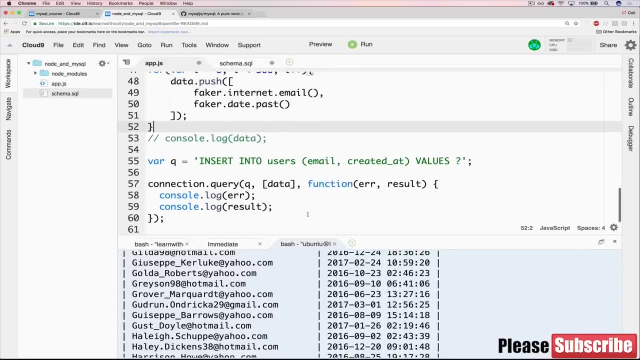 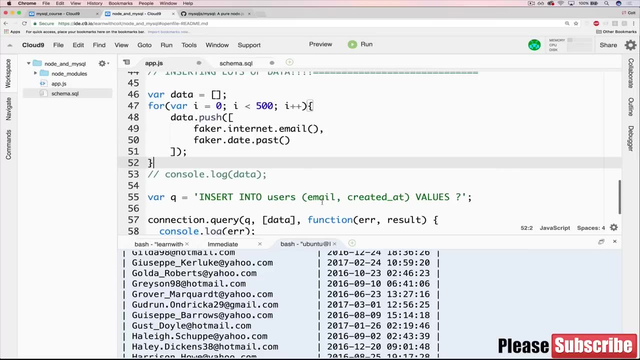 I'm aware if you don't know JavaScript, I can imagine it's quite intimidating, But hopefully the takeaway is not that you're a JavaScript genius that you could recreate this on your own, but more that you see that we're able to use JavaScript to insert or select from a MySQL database and that we can do things. 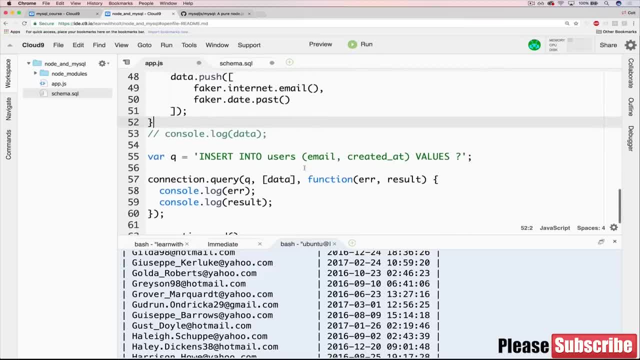 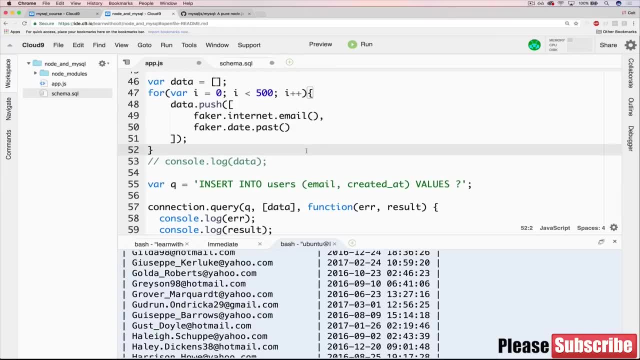 that we could do on our own, like insert a single user. but we can also do really powerful things that we couldn't do on our own or would take forever, like inserting five hundred users that are randomly generated with just a couple lines of code. 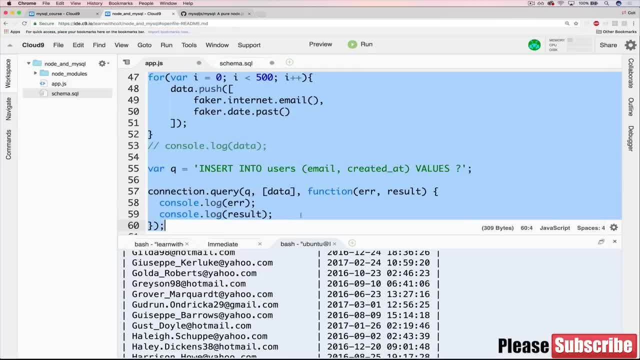 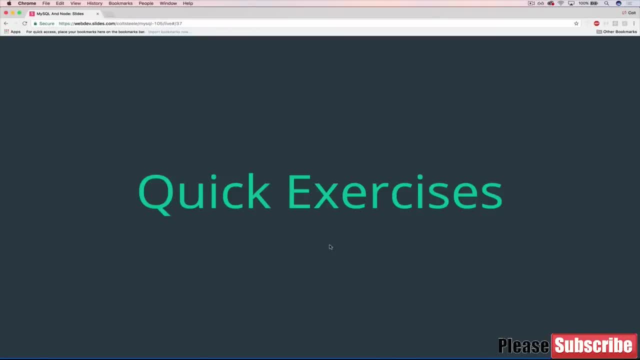 So this is really our first thing that we've seen that takes advantage of the power you get from using a language like JavaScript. Awesome, All righty. So we inserted five hundred users. It was kind of a behemoth of a section to get there. 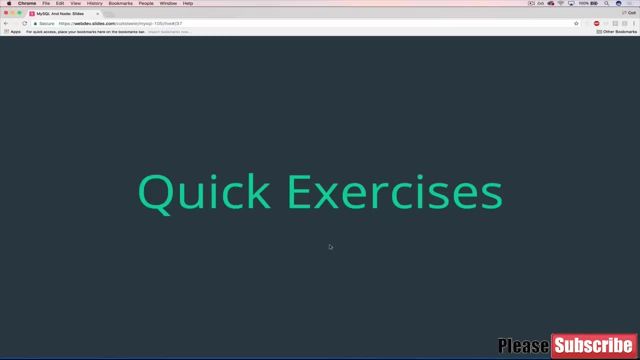 Lots of ground to cover, But now that we're there, we're back in our comfort zone. Hopefully we're going to have a couple of exercises. I know we have a lot of them, but this is cool. We have a lot of data now. where it was a single, you hit the return key once. 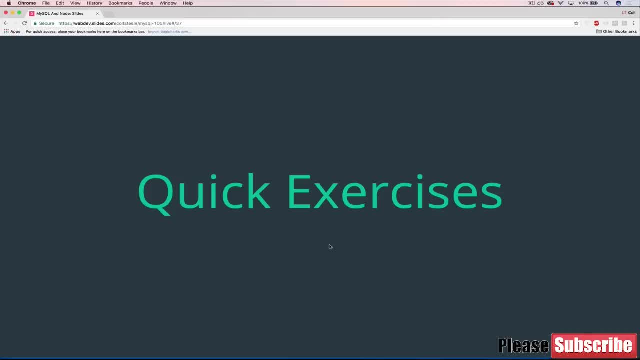 and you got five hundred users- much easier than having to copy and paste like 20 books. So we're going to play around with them. And again, your data is randomized, just like mine, So your tables and your results will look different, but the queries will work the same. 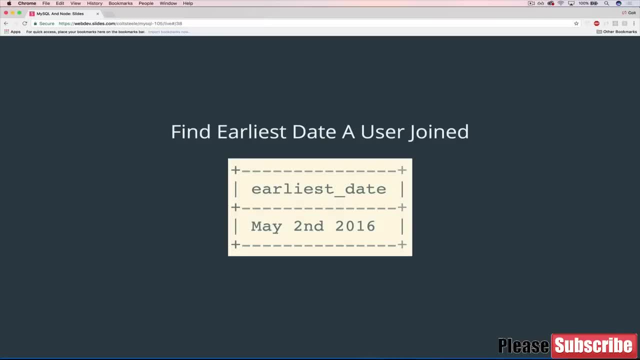 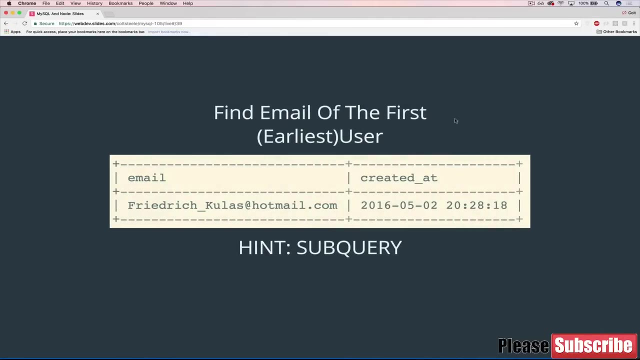 So here's the first thing: Find the earliest date that a user joined, and all we need to see is the date And also notice how I formatted it. Pay attention to that. So just the earliest date, and then the next problem: Find the email of the earliest user. 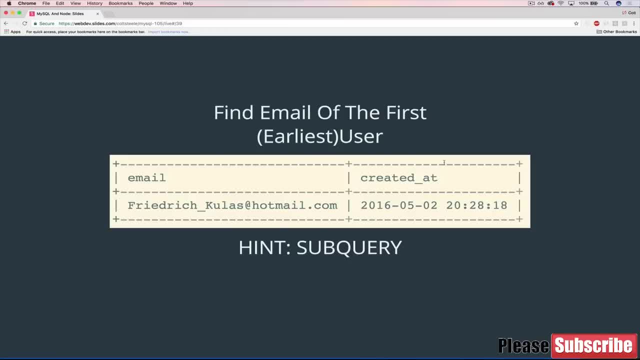 Now this one's tricky. Remember how we talked about this with Min and Max way back a couple of I don't know five, six hours ago, about how, when you use Min and Max, you don't just get the Min, You don't get the row itself. 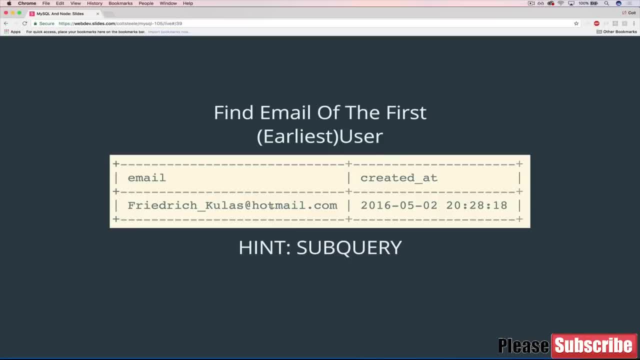 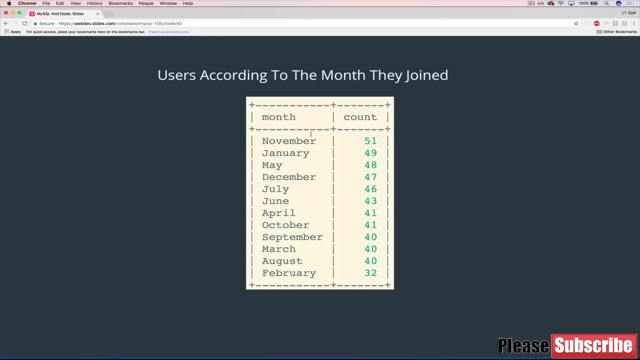 So we had to use a sub query. So the hint is: use a sub query to find the email That corresponds to the earliest user, Then take all the users, and I want to see a table where we have a month name and then the number of users joined who joined in that month. 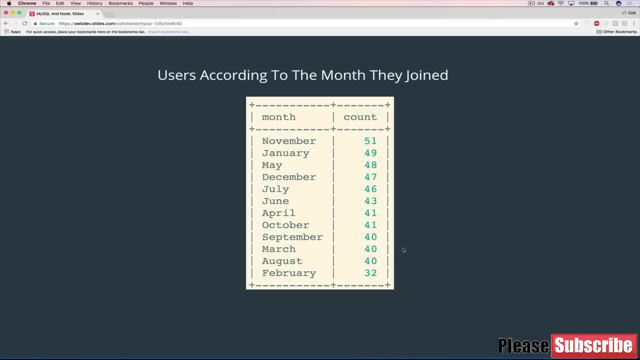 So it doesn't matter what year we have- some 2016,, some 2017, most likely. So we're not grouping by that, just by the month. So you have to figure out how you extract the month name from the date and then go from there. 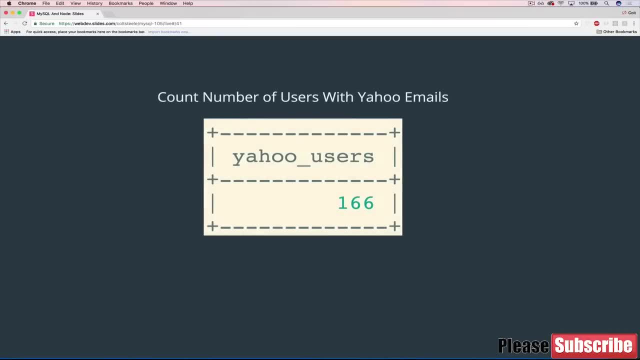 Also notice the order. Then Count the number of emails, or the number of users with Yahoo emails, And the way that you can determine that is just if their email ends with at Yahoo dot com. So how do you do that? Count them all? 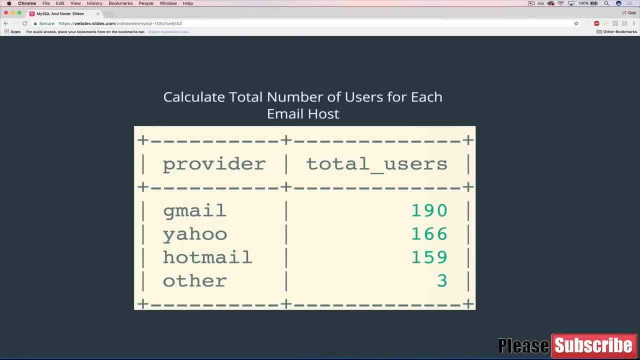 And then finally calculate the total number of users for each email host. And this one's a little bit complicated because you're basically going to be doing four different checks Going to say, all right, does the email end with Gmail? Does it end? 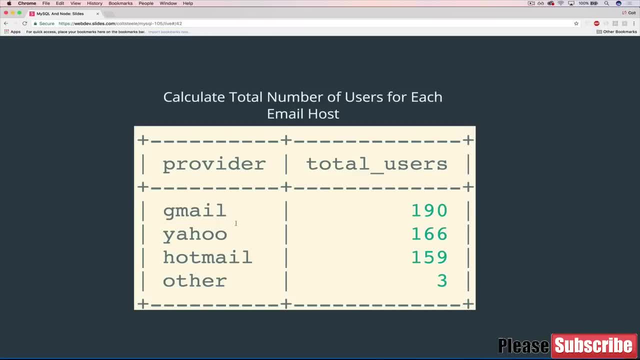 Does it end with Hotmail, And then you need to calculate how many each end with these. So it's a little bit complicated. That's why I left it for last. Hopefully you're able to get it. If not, solutions coming up in the next video. 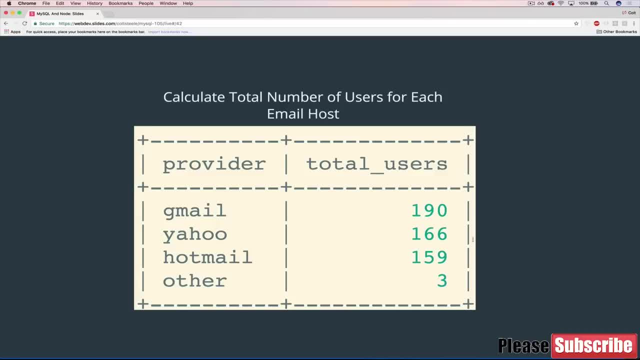 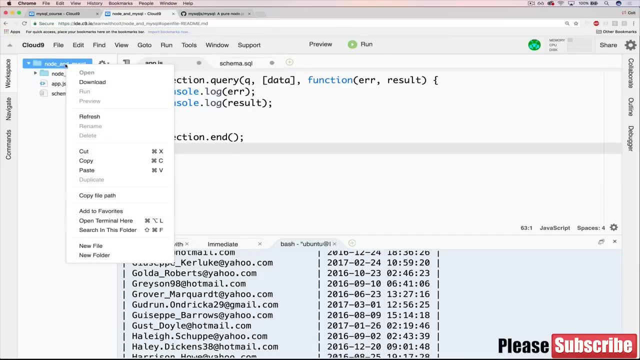 Just remember. your data is going to look different. Don't panic if your numbers are different. All right, I'll see you with the solution. OK, here we go. So let's first start off by just making a new file to work in. 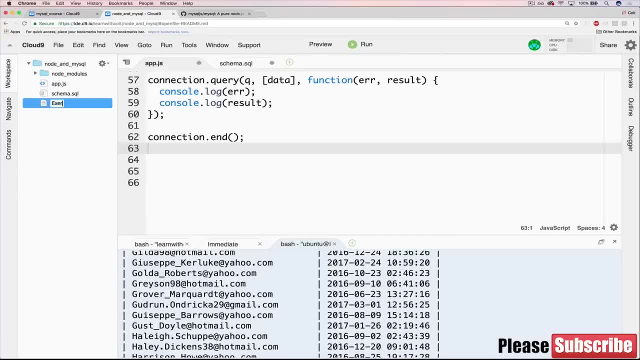 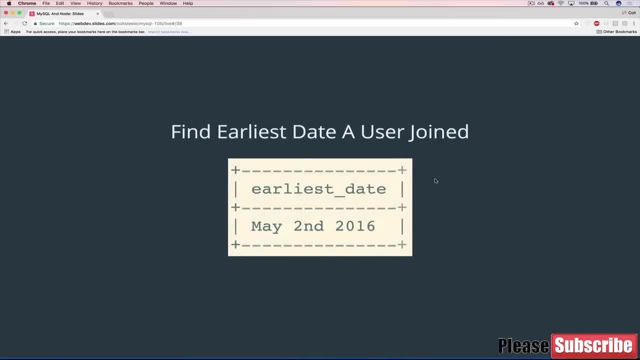 So we have some clean. We'll just call it exercisesSQL Now, just so we have a nice place to put the answers. OK. so our first one here: find the earliest date a user joined And we're not selecting anything except the earliest date. 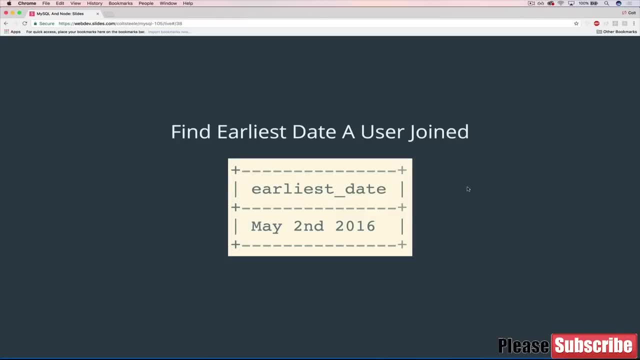 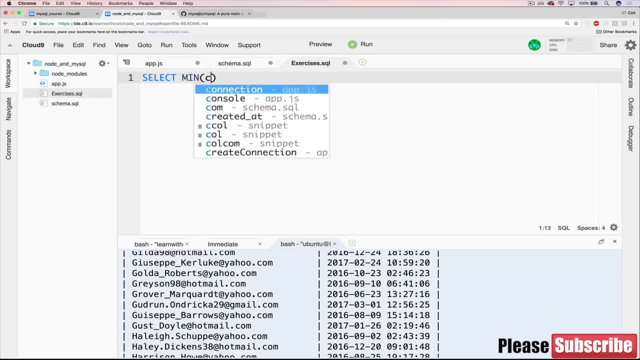 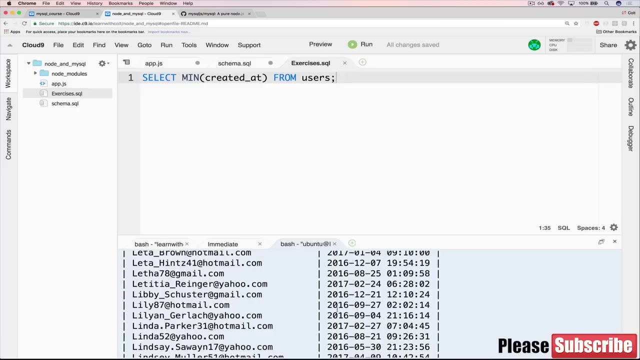 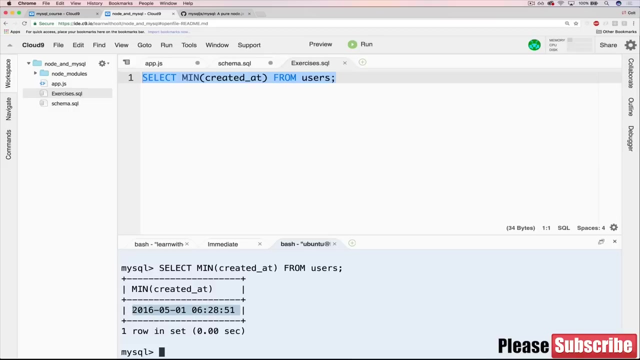 So all we need to do is take advantage of created at and use the min operator, the min function. So it's just a matter of select min created at from users and we'll save that. Copy it, paste it, And the one that I get here looks like this: 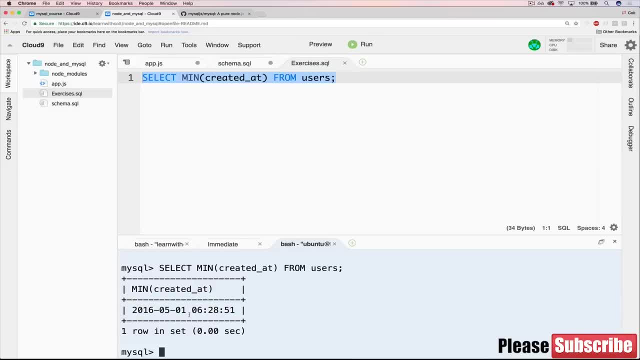 So 2016 501 notice says earliest date. So that's the easier part to fix And then notice the format. So let's do as earliest date first. That will make it cleaner. Then we need to format the date. So I'm going to put this on a new. 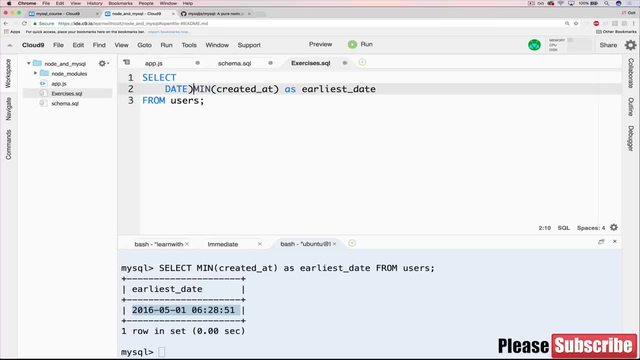 line and the way that we format, remember, is we use date underscore format. Think back to our date section. So we're formatting the result of the minimum created at, which is this, And we have a second argument, which is the date string, how we want to format it. 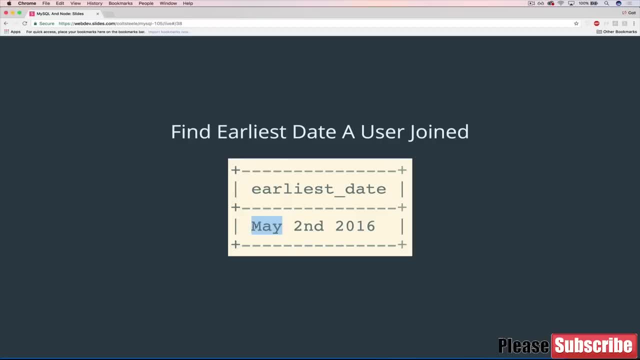 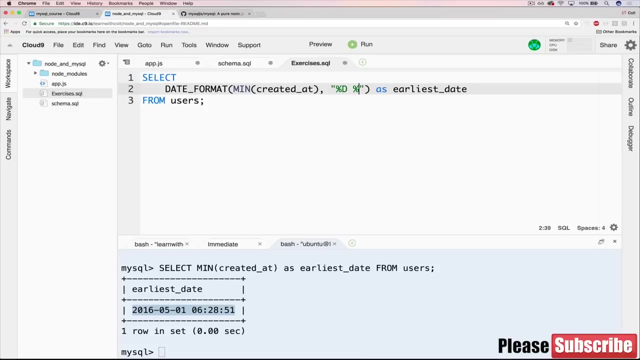 And the one I gave you had the month name, which I believe is capital M, And then the day with the suffix, which is, I believe, capital D, and the year for letter, four numbers, capital Y. So you need percent capital D, percent capital M. 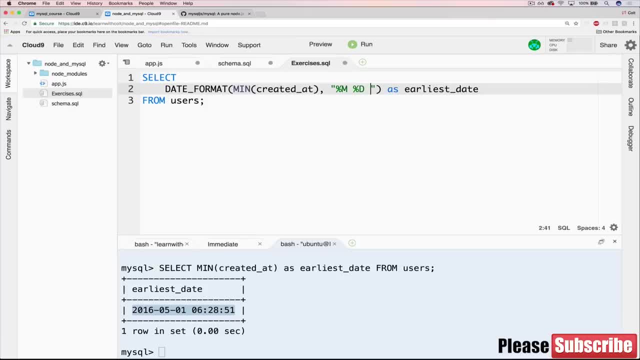 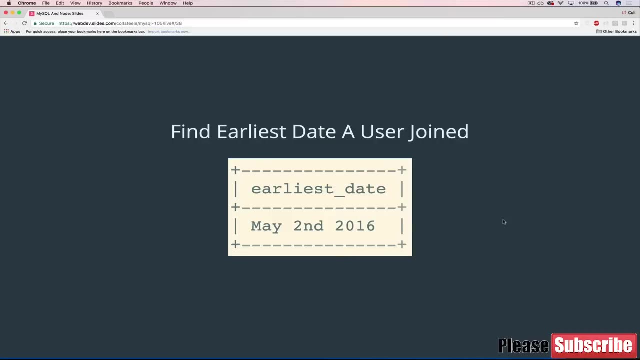 Nope, Backwards. Capital M percent capital D percent capital Y. Let's see, Oh, I have to copy this. paste it in And there we go, May 1st 2016.. OK, look, we're only a day off from the first data set that I added. 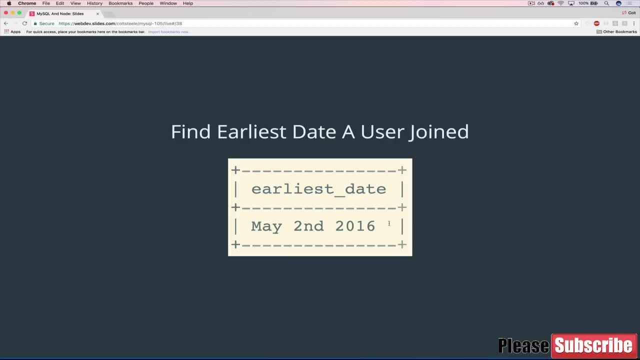 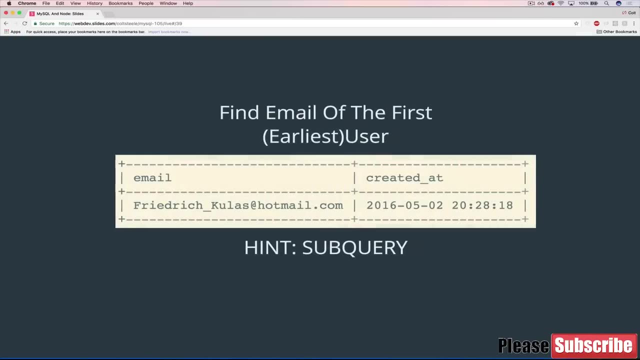 When I made these exercises, I had a different set of data and you just watch me rerun it, delete it all, create 500 new ones. So these will be slightly different than my answers. to next, find the email of that user, So the same one that we just found. this is the earliest date. 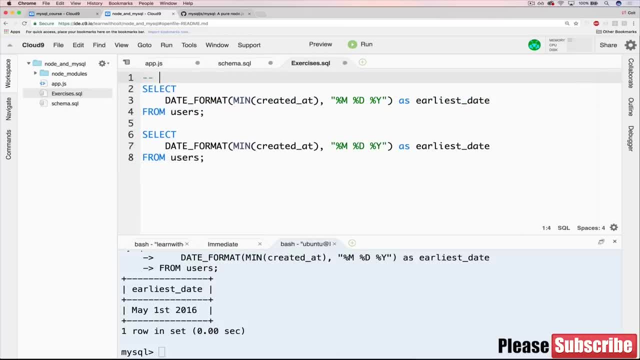 How do we find the email? So let me label this challenge one And this one. we have to use a sub query because basically what we're trying to do is: well, first we can clean this up a bit, We don't need to format this one. 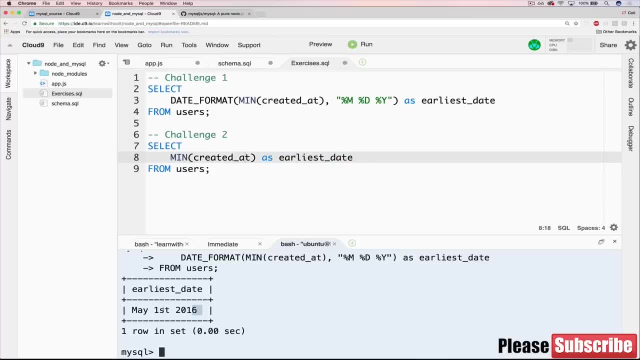 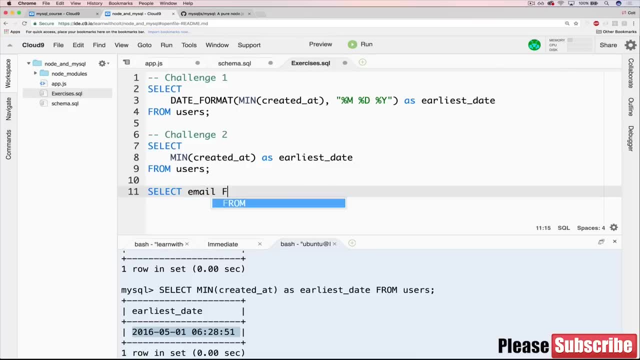 What we're trying to do is take this earliest date, which looks like this, And then we want to do a select. We'll do an email from users where created at is equal to that date. How do we find that user? So let's just do it manually. 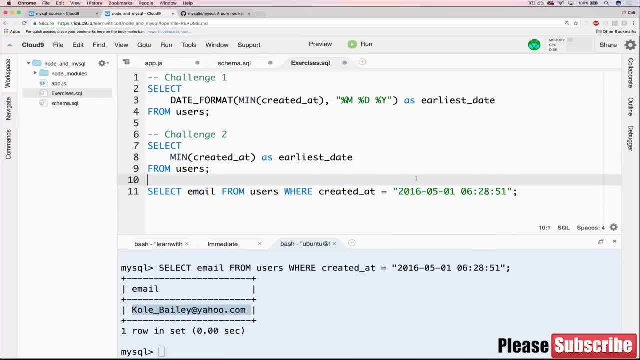 It looks like our answer is Cole Bailey at Yahoo dot com, so we can use a sub query to help us where all we have to do. we can get rid of this and say select email comma created at, or we could just say select star to make it shorter. from users. 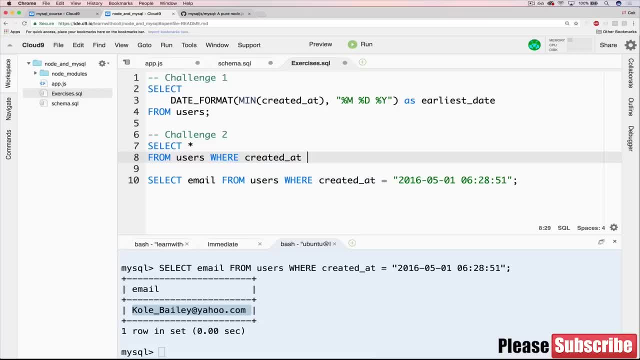 where created at equals. And then we have to do our sub query: Select men created at From users. so those parentheses that this is a query that needs to happen. So this is evaluated: What is men created at? I need my parentheses to work there. There we go. 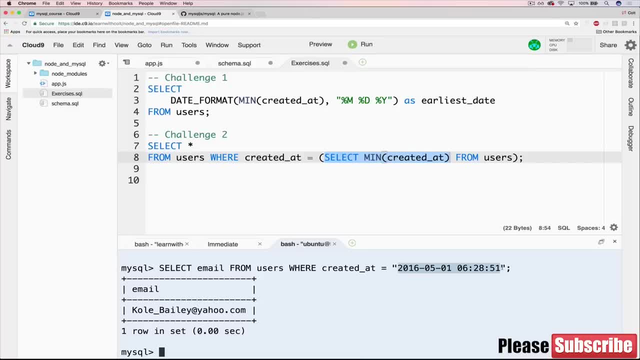 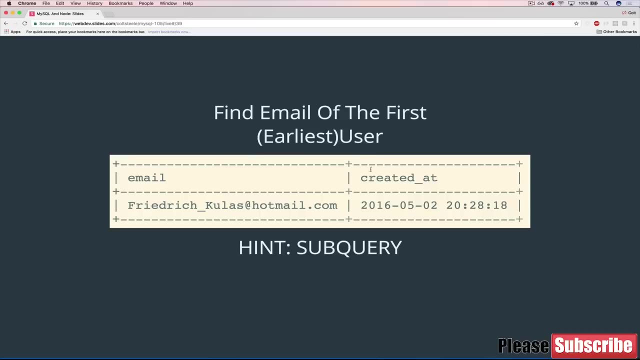 What is the men created at? Well, it's going to be this. So then, basically, this whole thing is replaced by that, And then we're finding users star from users where created is equal to that. So let's try it. There we go. Looks good. 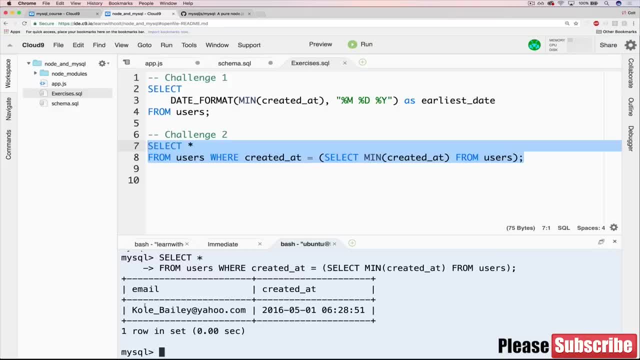 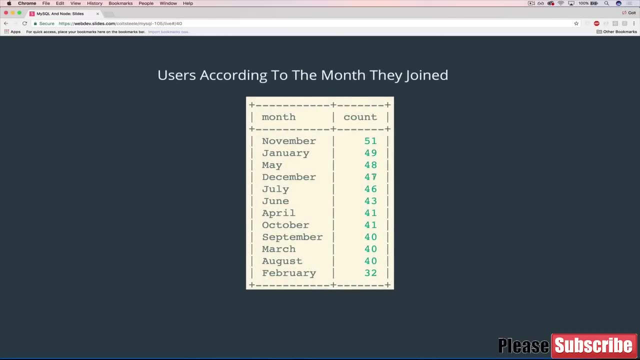 We've got email and created at. of course it looks different, But this is the correct answer, called Bailey, And we saw that because earlier we just manually selected it based off of that date and it worked perfect Moving on. So we're taking every user, taking their created at date and then we're extracting. 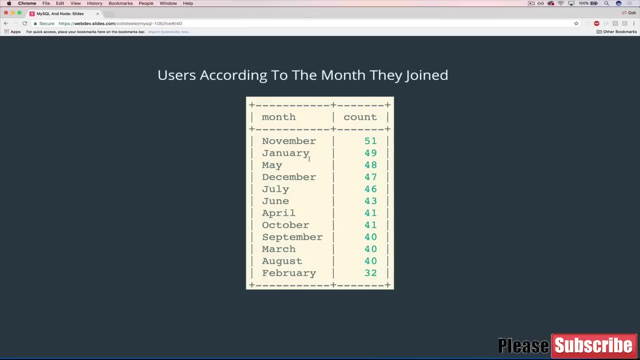 the month name from that date. whatever the month is combining them all, We're grouping them and counting how many exist. So how many users signed up in November? In our case, November was the highest, And then we're sorting as well. 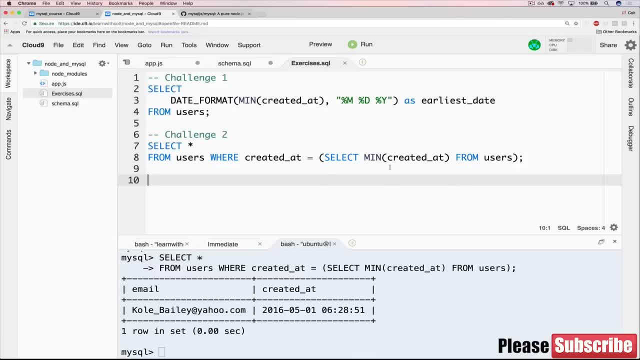 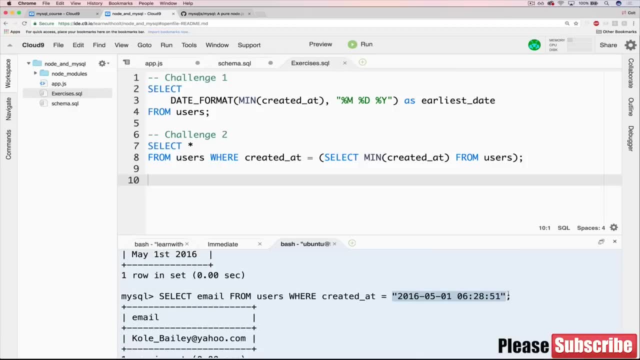 So let's start by just extracting the month name. So if we were to take a date like: where is that This one, right here, How do we get the month name from that? Because if we just do select month of that, it gives us a number. 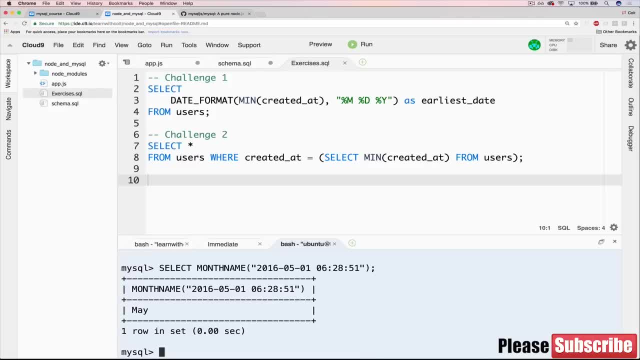 So what we can do instead is month name, and that gives us May, So we'll start with that And we'll do select month name of created at from users And we get 500 different month names. Well, there's only 12 different ones, but 500 rows. 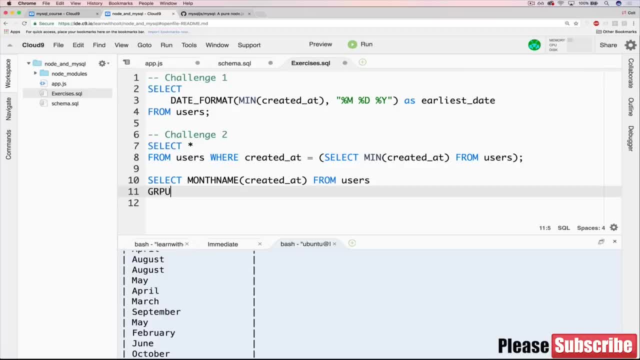 So, then, what we want to do is a simple group by- and let's just give it a name like as month- and group by month instead, Rather than retyping that whole thing. Okay, So now we have 12, assuming that we have a date in every month of the year. 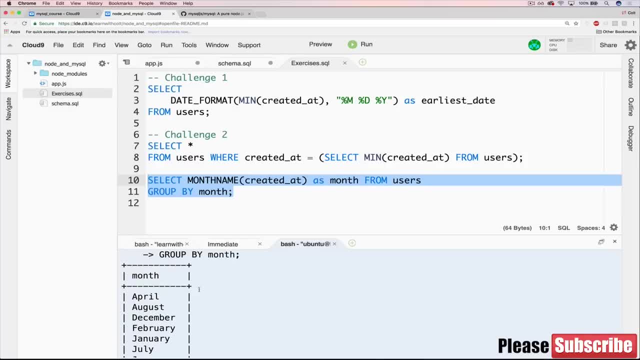 which we probably do if we have 500, but we don't see how many there are. So then we need our second field, and our second field is count. We just do count star, just like that, And here we go Almost there. 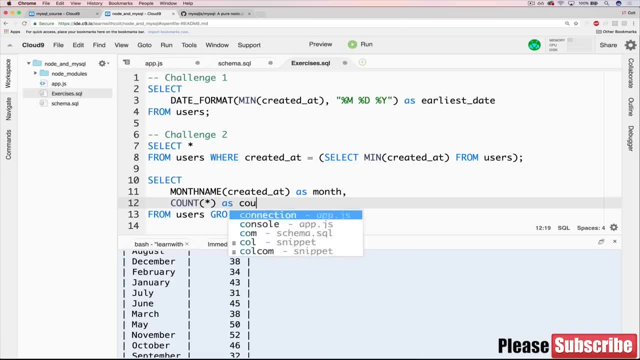 All that we need to do. I believe I gave this an alias of count- And then we also want to order by count And we want it to be descending. Let's see if it works. There we go November, the highest count as well, with 52,. 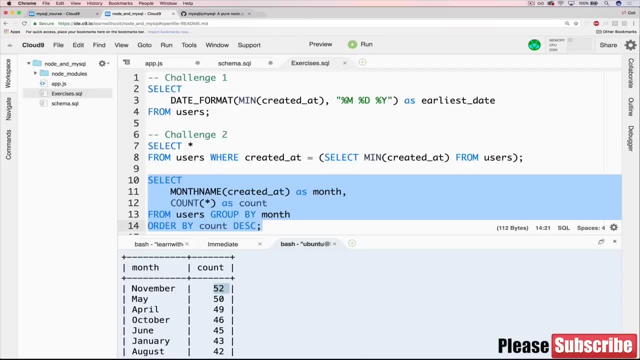 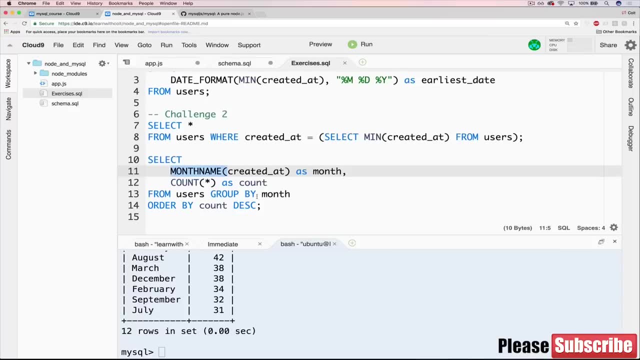 although it diverges. January was first or was second, in my case May and then April. All right, So we use this month name and we group them based off of that month. You could also just replace it with this, but it's easier just to type month. 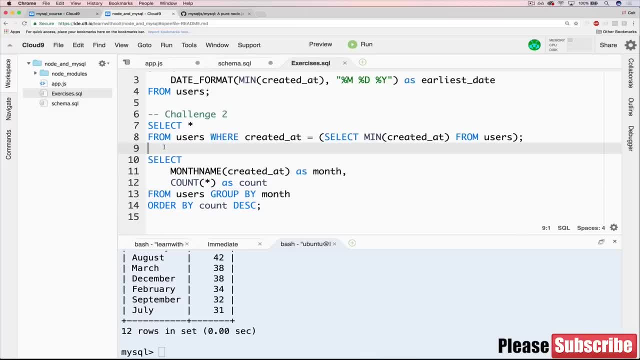 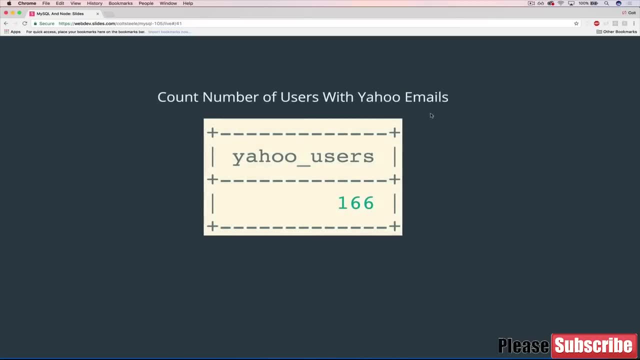 And then we're grouping them, counting them and ordering them. Let me just put a note that this is challenge three, Moving on Challenge for count the number of users with Yahoo emails. So for this one it's a bit of a throwback. 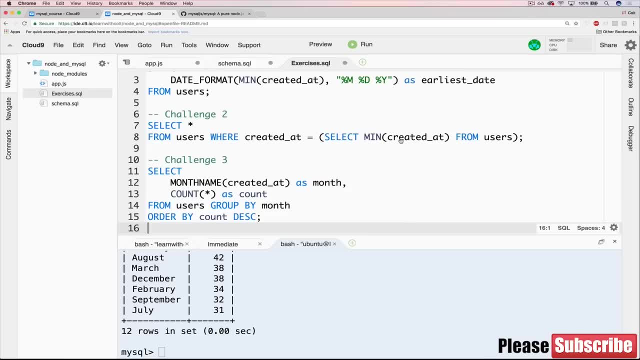 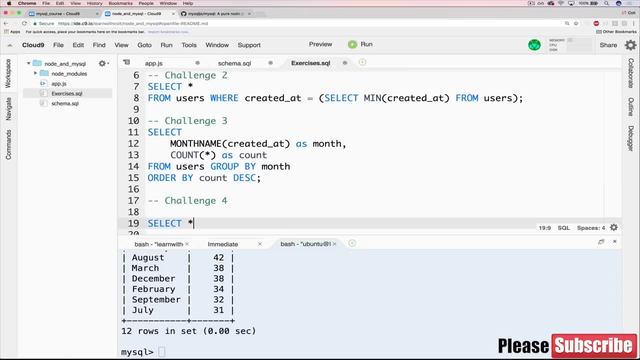 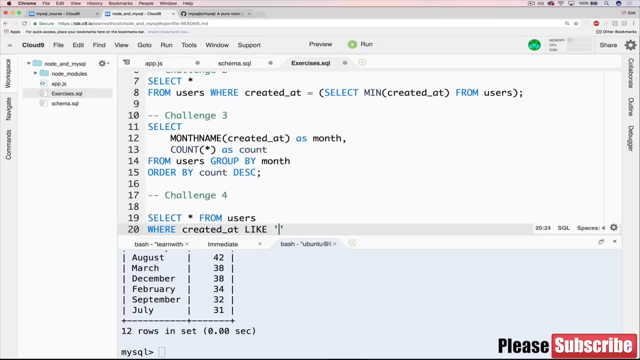 All we need to do is use like to figure out which emails have Yahoo in them. so we'll do a challenge, for Let's do a select star from users where we just need to say we're created at like And we don't just want to say Yahoo, remember, that's only going to find. 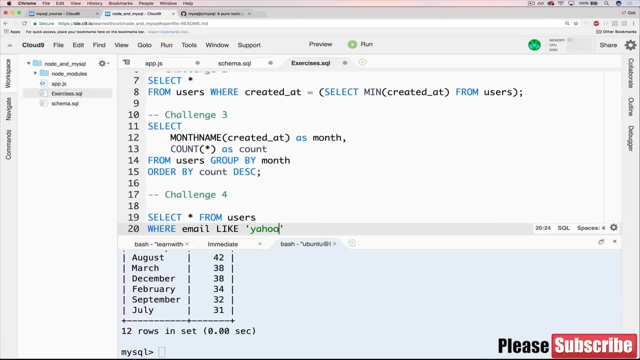 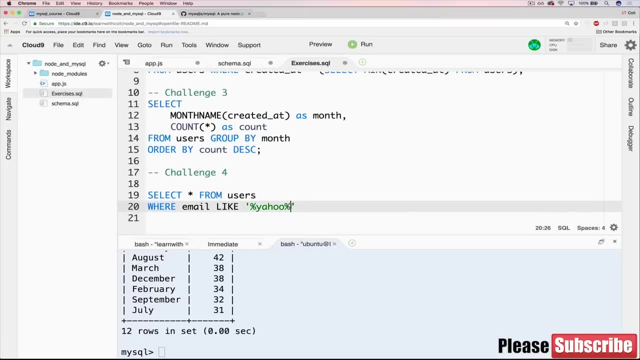 And what am I saying? Created at where email like Yahoo. We don't want to do that because that's only where email is exactly Yahoo. So we need these, The placeholders, But we can improve this a bit, Because this would match anything that had Yahoo in the string anywhere. 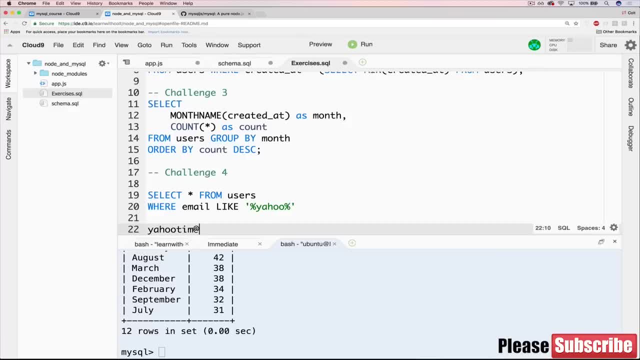 And we could have someone's email, be you know, Yahoo, Tim, at Gmail dot com. Or maybe someone's last name is Yahoo or something Yahoo's. So we don't want that. So all we want to change is: we'll do at Yahoo dot com. 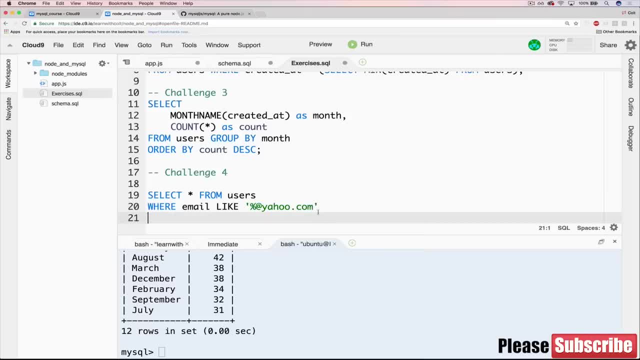 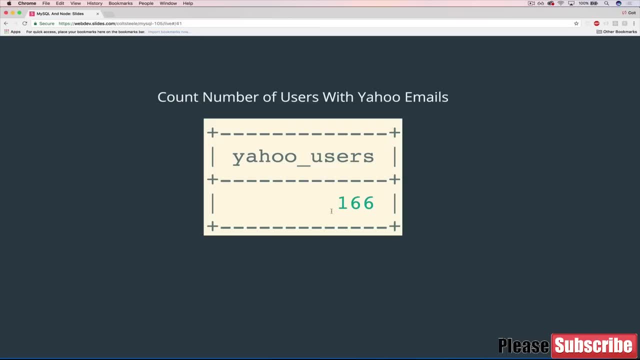 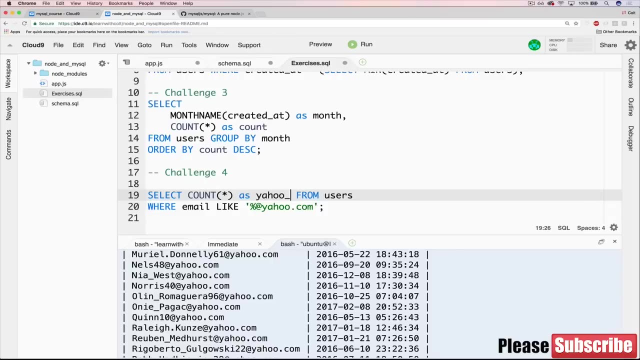 And this will guarantee that the string ends in at Yahoo dot com. So now let's take a look. Here we go. These are all Yahoo dot com emails, And then all we wanted to do is count how many. So rather than selecting star, we'll do select count star as Yahoo users. 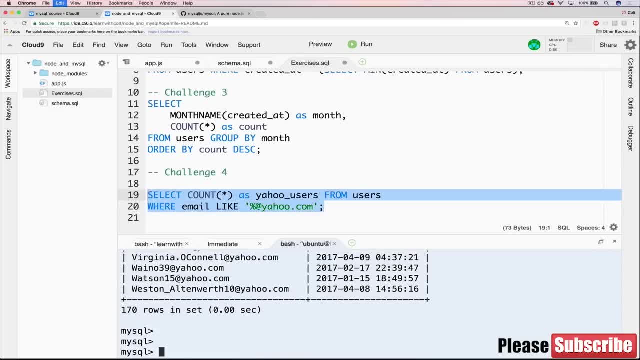 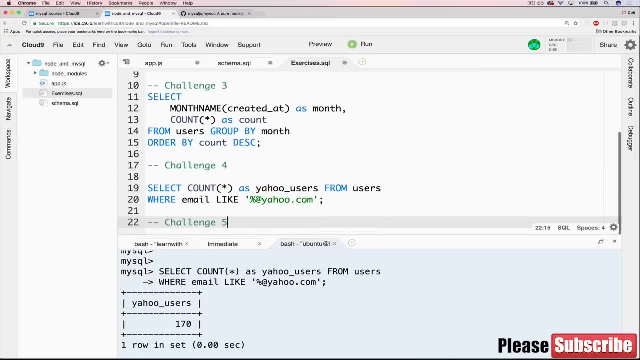 I think it's what we called it- From users where email is like Yahoo, and this time there's one hundred and seventy. And finally, challenge number five: calculate the total number of users for each email host. So this one involves using like. 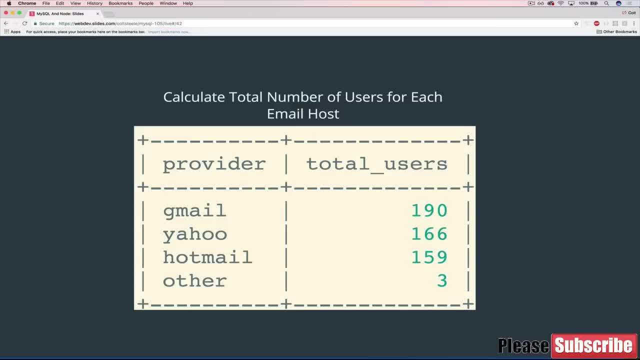 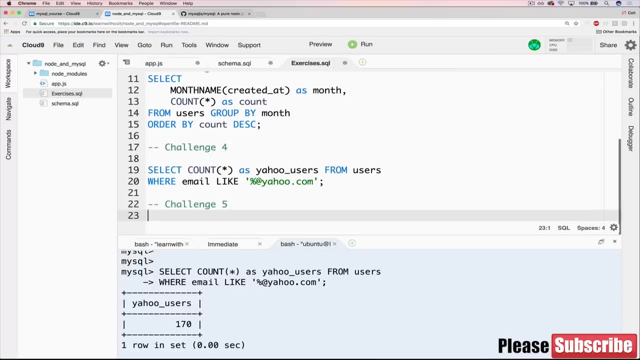 along with a case statement. it's a little bit complicated. So we're doing the same thing where we're counting the number of users, but we're doing it dependent on the provider. So we're going to have a case statement. so we'll just start right off with select. 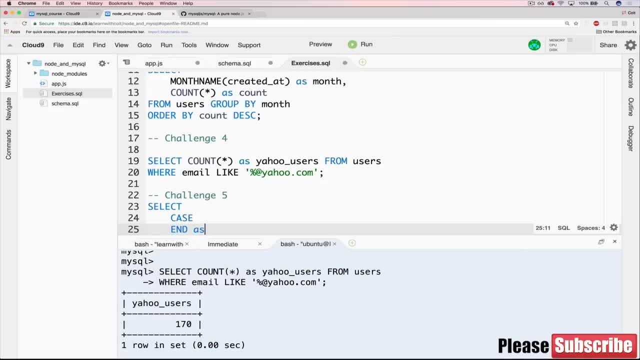 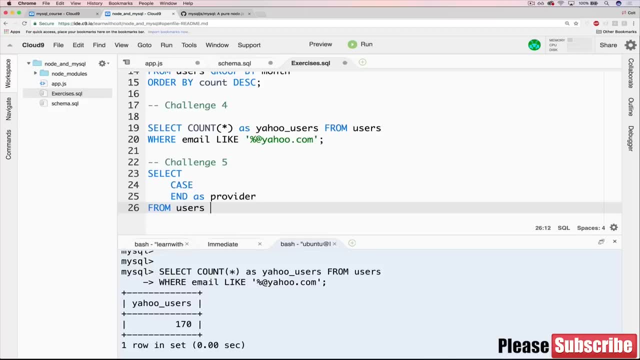 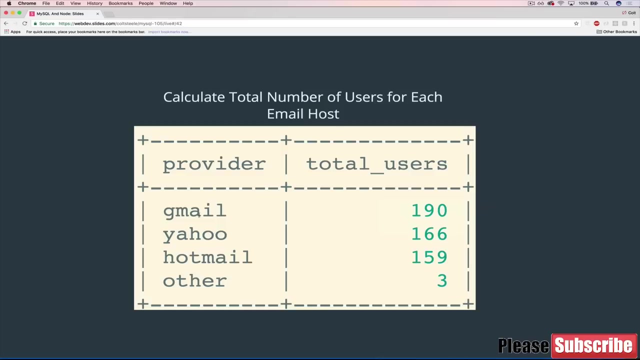 We'll do case and I like to do my end as- and I think we called it- provider. Yep, So we'll start with that And we'll do from users. And what is our case? Well, we can start with This. Yahoo, one will say. when email is like Yahoo, then provider is Yahoo. 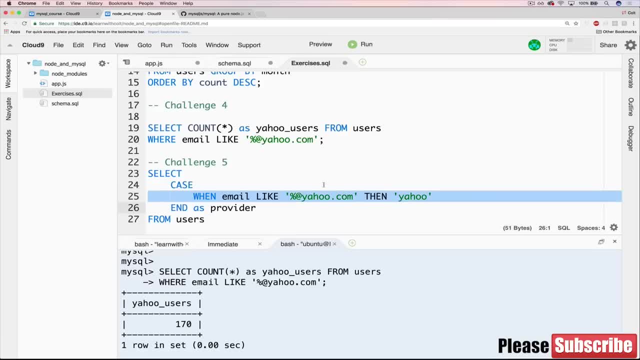 Right, So we'll do the same thing. Just basically copy this And say: when email is like at Gmail dot com, when it ends in Gmail, then Gmail. One thing I should note: there is a kind of nicer way of doing this if you are familiar with regular expressions. 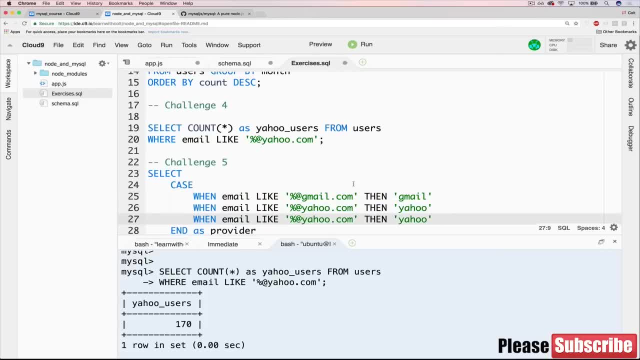 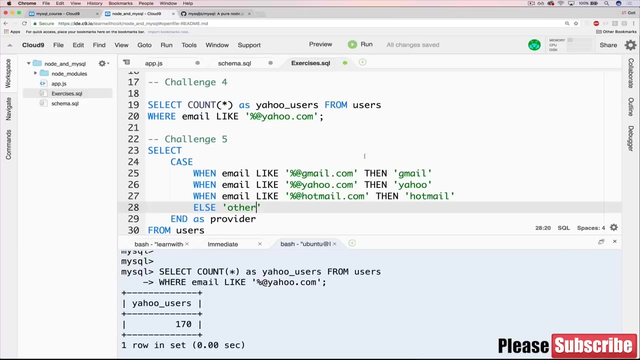 That's out of the scope of this course, But if you do know it, you can get by with that. So we've also got Hotmail, Then Hotmail. There we go, OK, then finally we'll have our else, which will just be other. 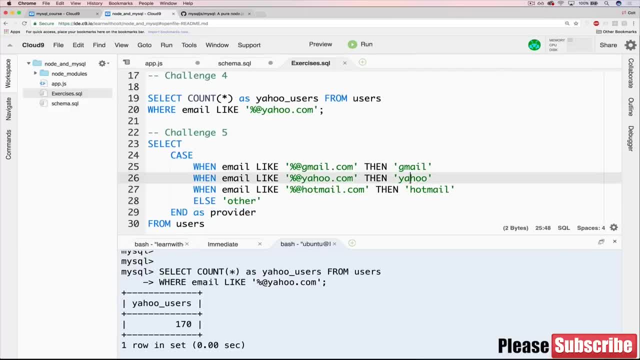 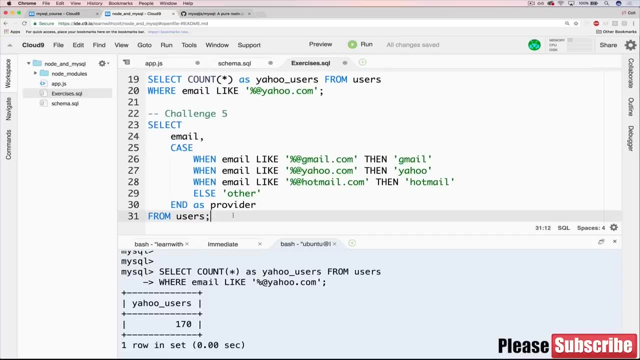 So we have this provider field, now a column that will have Gmail, Yahoo and Hotmail or other. So let's do email comma case so that we can see the email side by side against what we pulled out of it. So we got 500. 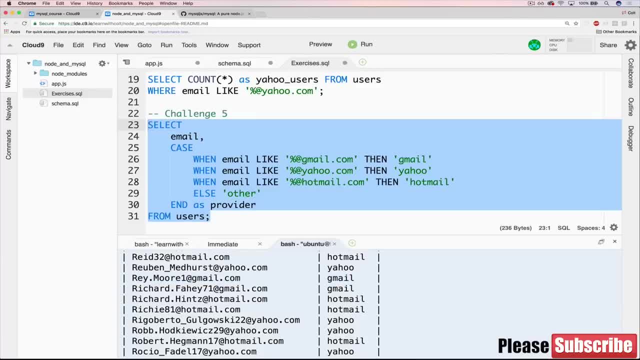 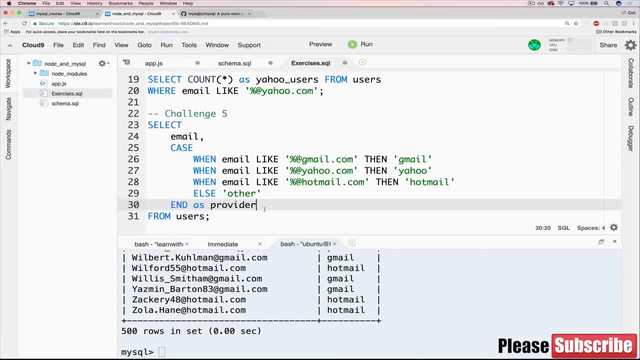 Let's take this one: Ray dot, more one at Gmail, We get Gmail. Ruben Medhurst at Yahoo- We get Yahoo. Perfect, So now it's just a matter of grouping them together and counting so we can get rid of email. 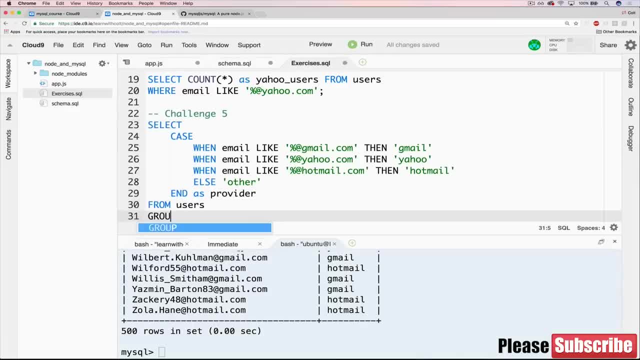 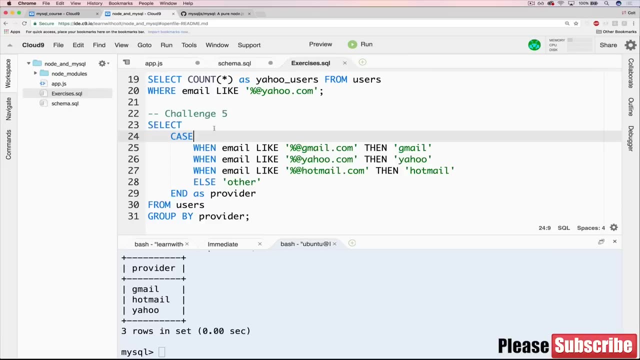 We don't need to display it. Then we're just going to group by provider, which is what we just created. So let's start with that. Cool, So we're grouping them together. It looks like we don't have any others. in this case, 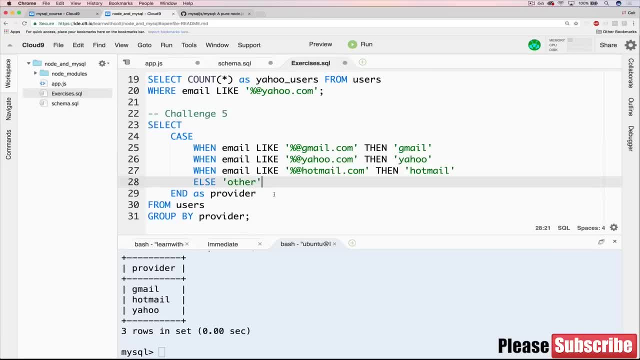 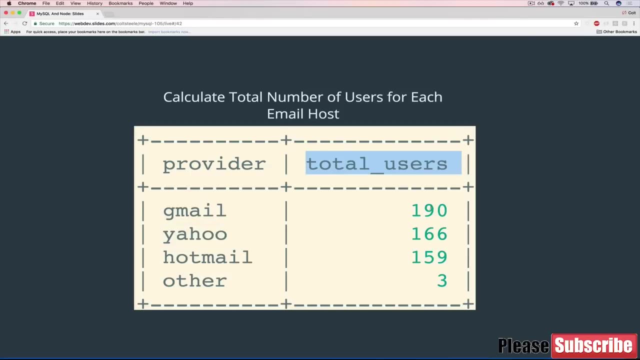 We're going to group them And then, finally, we're going to count. After our case statement ends, we add a comma count star, Copy paste And there's just a small discrepancy, which is this is called total users. Also, this is sorted very easy to change. 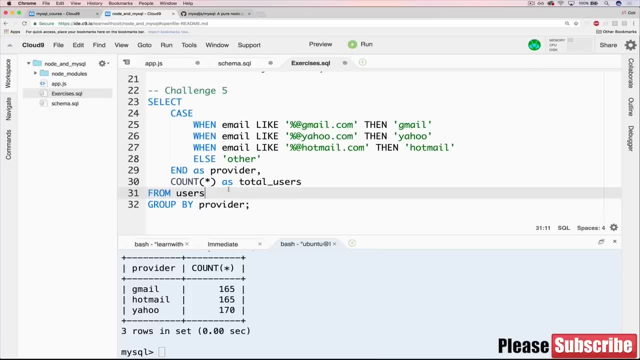 Call it has total users. I like to capitalize that actually. And then finally, well, let's just make sure that that works. to start Great, Now we need to sort it order by total users. If we do it this way, You'll see that it's ascending. 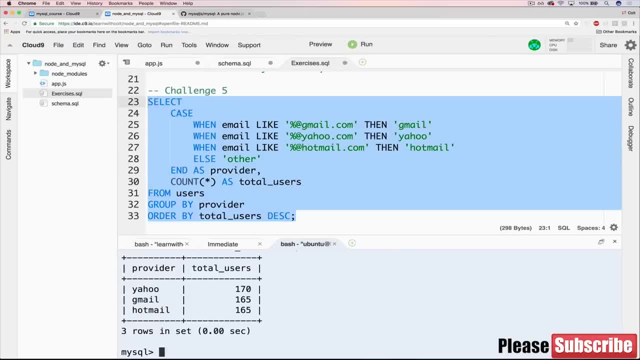 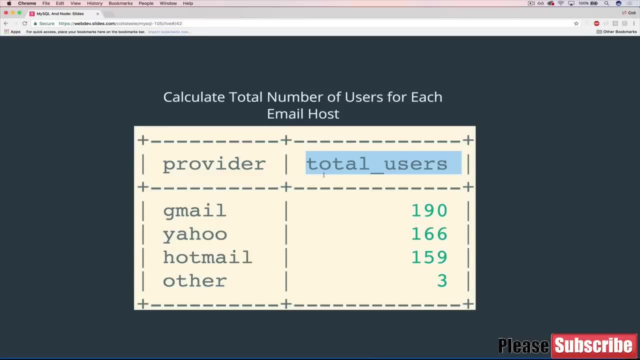 We want to do descending, All right. Now we've got all the providers on the left and their total number of users- Perfect, All right. So hopefully you enjoyed That chance of working with more data that isn't hard coded in some of its. 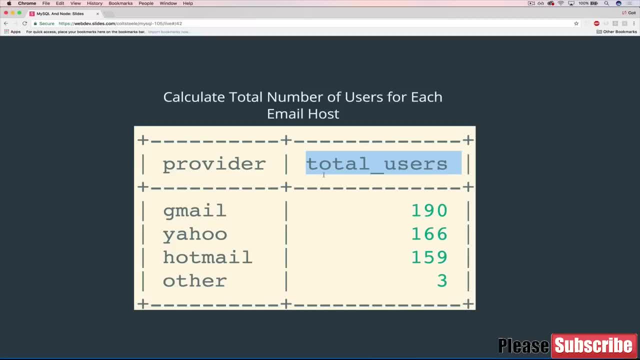 dynamic, all of its dynamic 500 plus users. Next up in the next section, we're finally going to connect the database we just created, which is filled with all that seed data, And we're going to connect it with a Web application and figure out how to get those to talk. 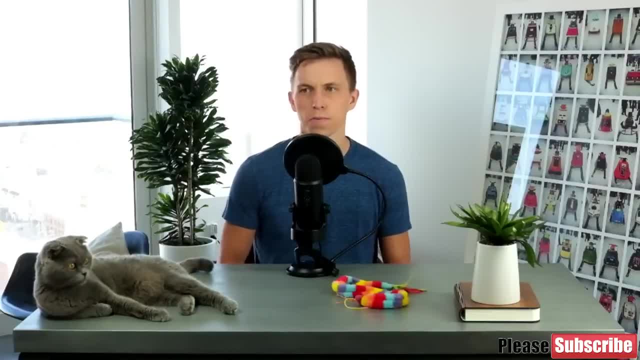 All right, We made it. This is the section that a lot of you probably have been waiting for. It's where we connect my SQL not to just a random node file, but to a Web application, Which is really just a random node file that has some other code in it we haven't seen yet. 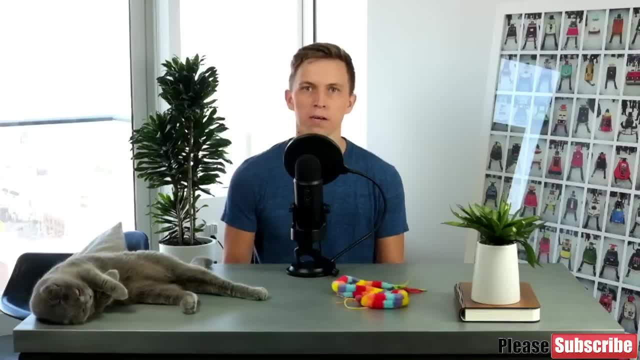 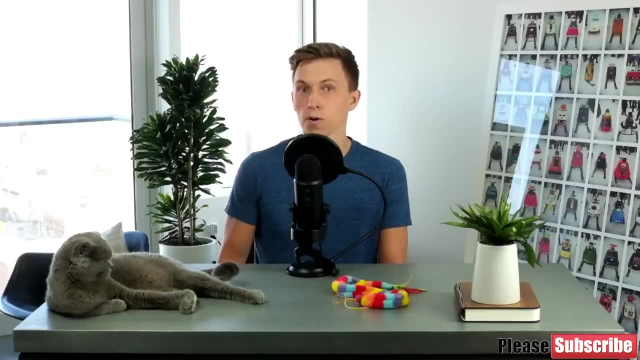 But that's what we'll see in this section. So we're going to build a very simple app that serves as sort of a mailing list for a startup. slash Colt C? U L T, not C? O L T or Colt. It's very hard to say. 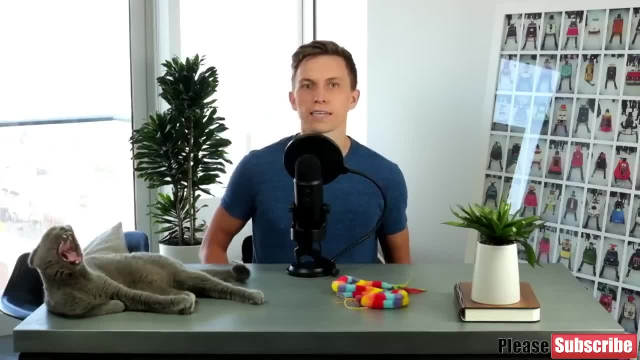 but that's where we're going to build a mailing list application that you know we could collect emails before we launch a product or something, or collect emails before the world ends, or whatever we're worrying about. So we're going to see how to do that. 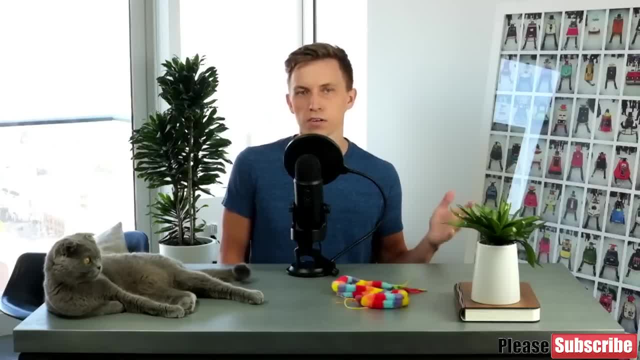 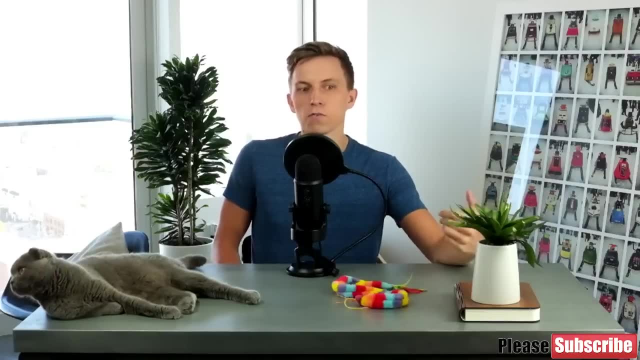 In this section it's going to be mainly a code along, So it's going to function. really. I'm going to show you something and you'll do it yourself. And I'll show you something else and you'll do it. There's not going to be a ton of new content as far as my SQL is concerned. 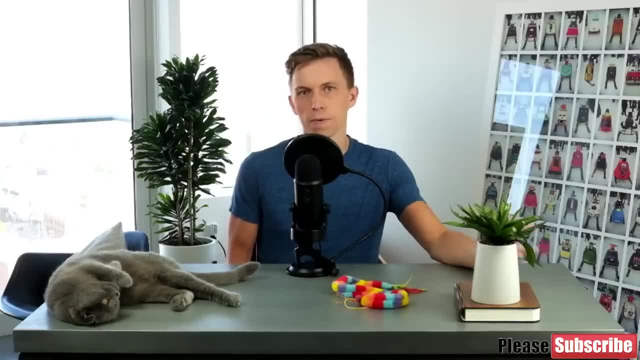 Really none. It's really all the auxiliary stuff that goes into a Web app. So if you don't know anything about Web development, I should preface this by saying there's going to be a lot of stuff here, And this is one section right. 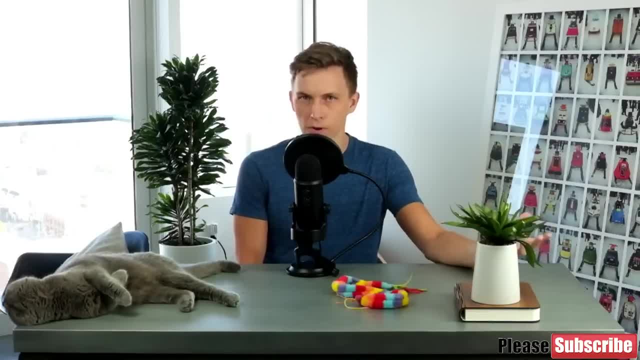 This could be a whole course on Web development. In fact, some people have- I've built courses on Web development. This is not a course on Web dev, So it's an hour or so of content, not 40 hours of content. 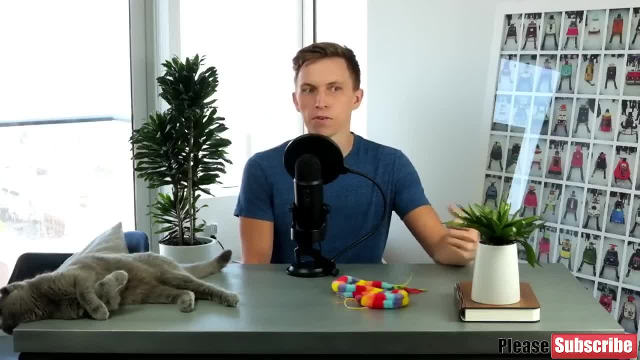 So don't get overwhelmed, Just follow along and build it. If you are someone who knows Web development, some of this may seem a little bit slow for you. For example, when I'm talking about HTML and CSS, feel free to skip. I mean feel free to skip whenever you want. 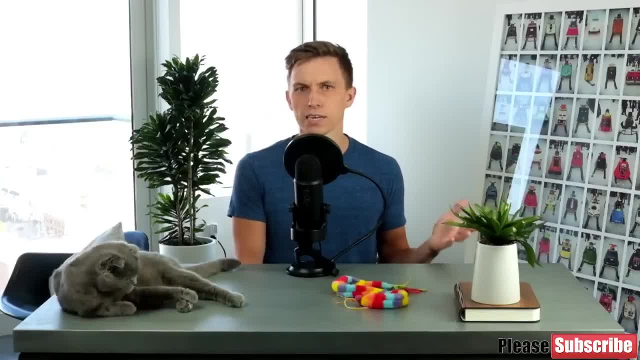 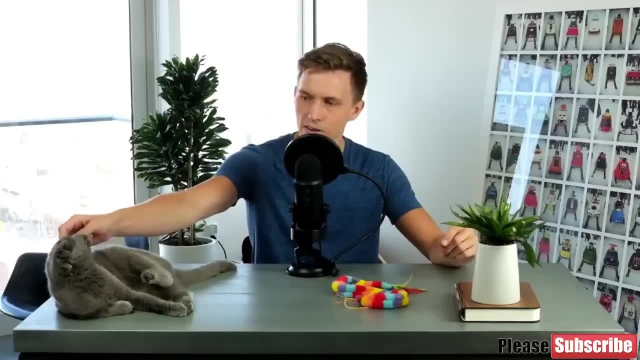 But in particular those sections. So that's pretty much all I have to say here. Congratulations on making it to this point, Very exciting. Hopefully We're going to see how to make an app. Blue's very jazzed about it, aren't you Blue? 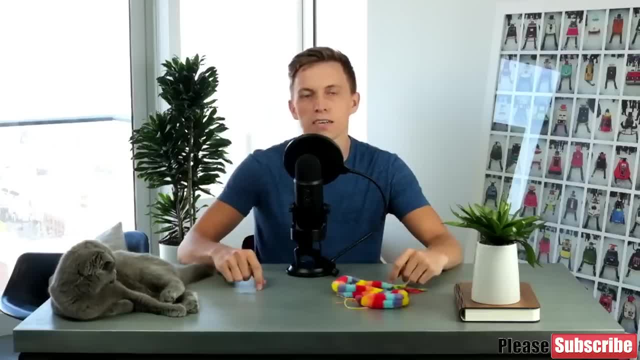 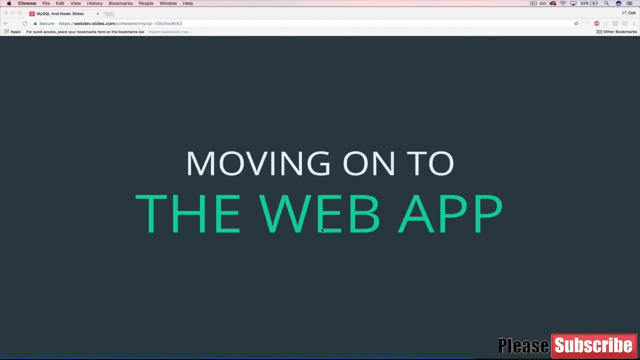 Blue. That's about the most excited she ever gets. I miss dogs. Hey, welcome back. Very high energy because we're moving on to a very exciting portion of the course. We've now seen how to take a database in MySQL everything we know. 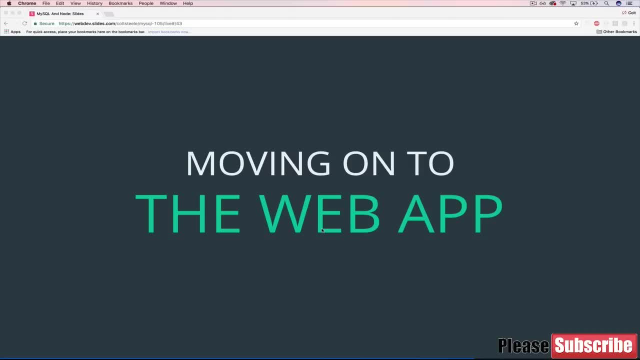 and combine it with a node file, a single file. that doesn't do. I mean, it depends on your impression of it. it doesn't do a whole lot, It just inserts. But it inserts 500 things, which is pretty cool. 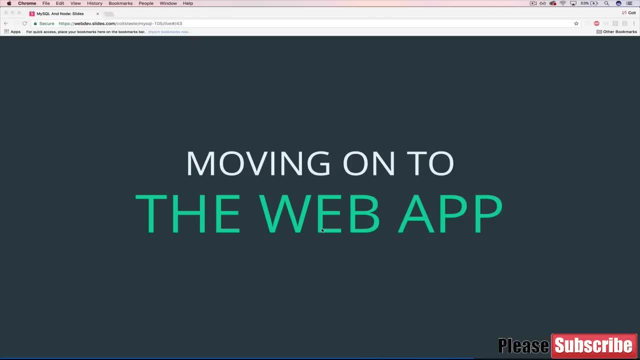 And they're all randomly generated. But that's not an application. that's still useful for our application. We'll be able to use that. just to recap The whole reason. we're doing that is so that when we start up our application we have some data in there. 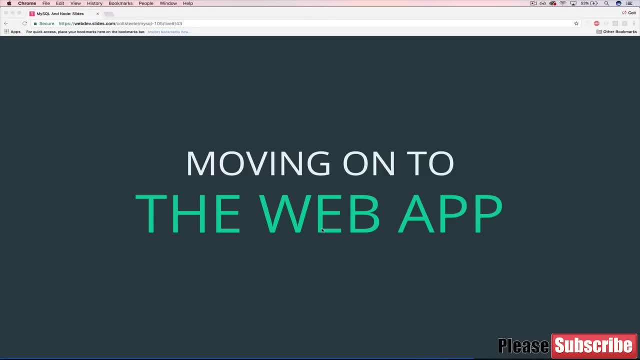 We have something to work with, rather than totally empty database or something that has two users. We have 500 realistic, randomly generated emails and created updates. OK, So we've done that. We have that. Now we're moving on to the web application portion. 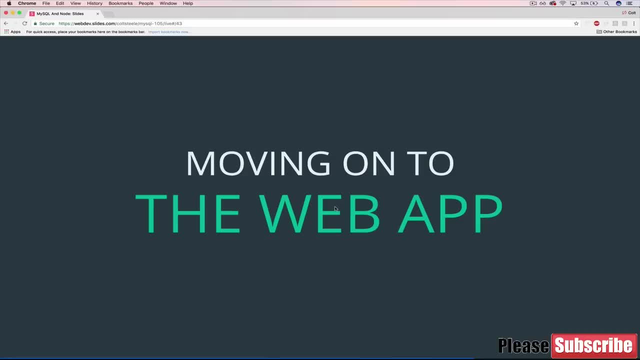 So remember this is join us, our mailing app or waitlist app, where there's a nice page with it looks styled, It's nice, It says join us. in big letters, It says how many users have currently joined And there's also a guarantee: 100 percent. 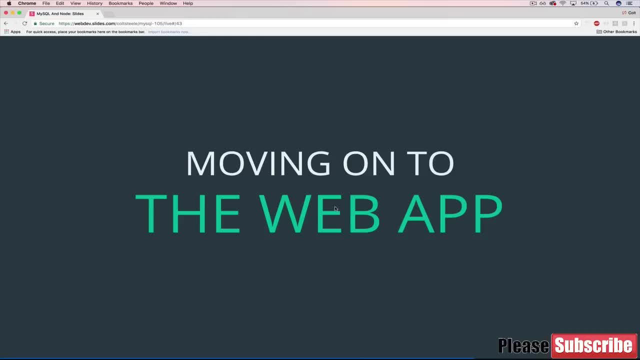 It's not a cult. And then there's a form at the bottom where you can actually enter your email to join the list. So we have to get there. We're going to start with the basics of a web app, So, just like we had to start, 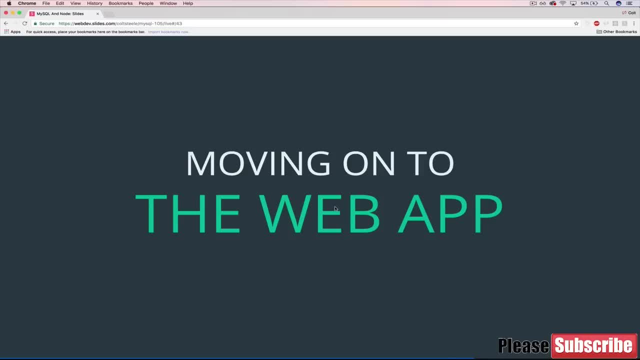 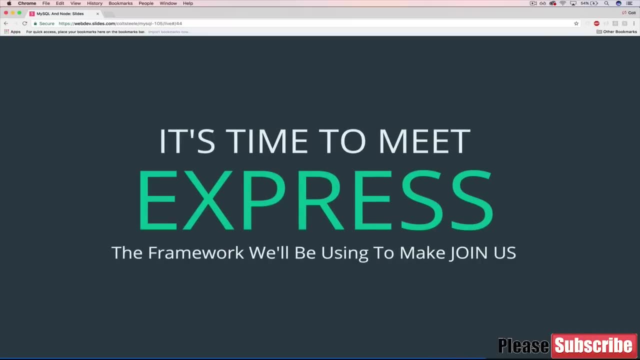 with the basics of Node. we're now starting with the basics of building web applications. OK, that brings us to something called Express. So if you've taken my other course, or if you're familiar with Node and you've used it in any web development capacity, you've probably come across the framework Express. 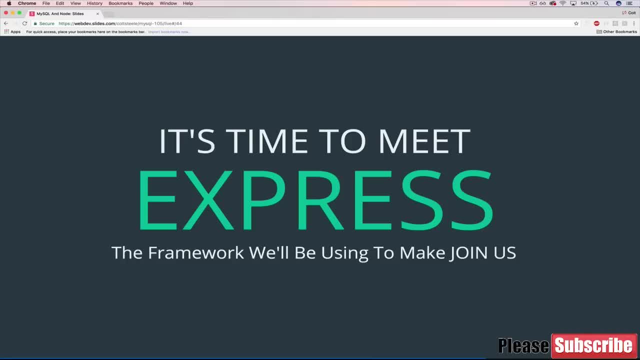 It's a web development framework. It helps us make applications faster. So if you're not familiar with frameworks in 10 seconds, what they are are tools libraries that are a bit more complex, a bit more controlling of how you write your code. they dictate things for you. 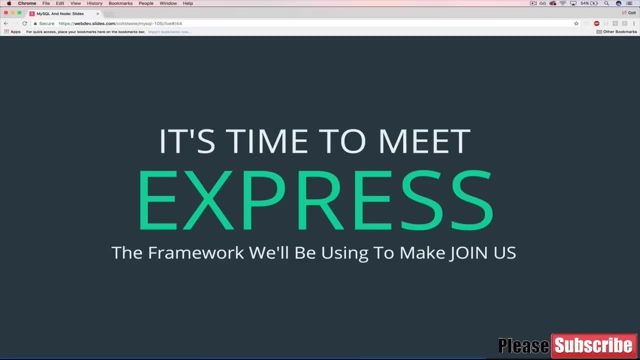 You play by the rules, but they help you make things faster. So a web development framework helps you make websites faster. There are iOS or game development frameworks that help you make games faster. So they kind of limit your freedom a bit but they empower you because they speed. 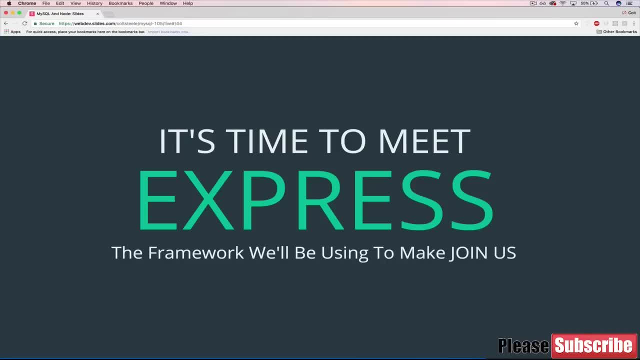 you up and they let it. they let you focus on the things that matter. So, with all that said, Express is very simple, a lightweight framework. What it allows us to do is, once we install it and include it in a file, we can very quickly make a web application. 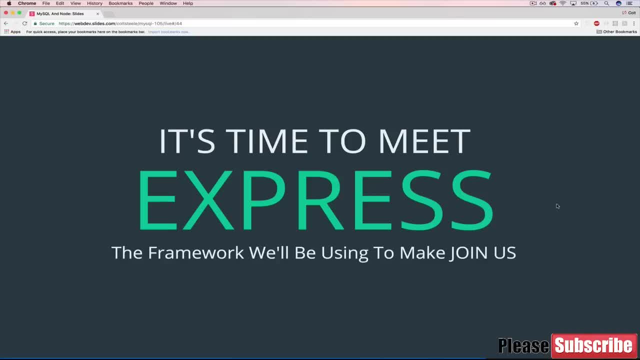 So something like Faker is a package that allows us to quickly get random data- a very small kind of feature that's it's useful, but it's a small thing. Express is a package that when you use it and install it, it does a lot. 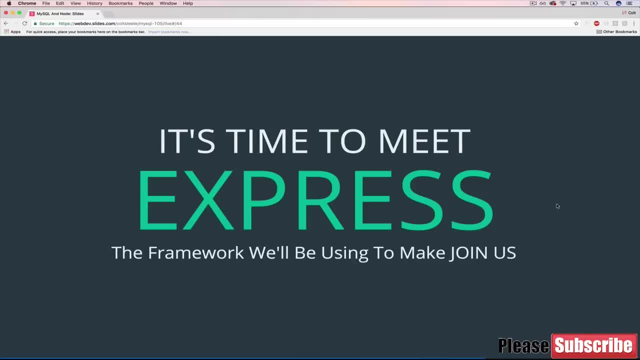 It sets up a server for you. It listens for incoming requests. It figures out how to respond to requests. It handles HTML and CSS and, responding with that, It figures out how to parse a response body. All these things We'll go into, but it does a lot. 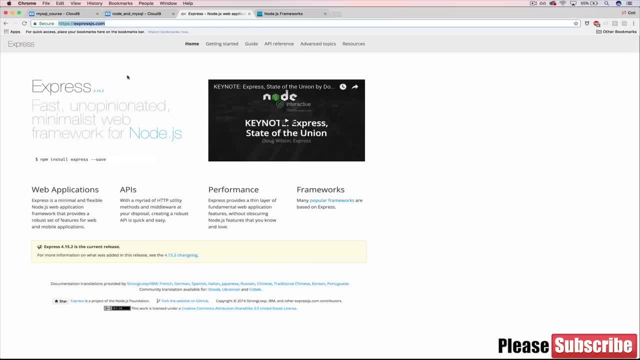 So let's take a look very quickly at the documentation: ExpressJScom, A fast, unopinionated, minimalist web framework for Nodejs. As you can see, you can just install it. NPM install express. We'll talk about dash, dash save in just a second. 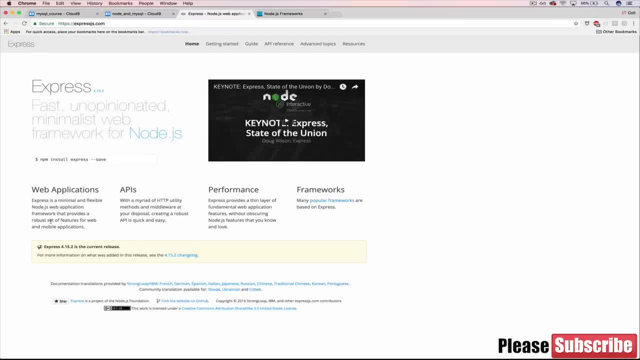 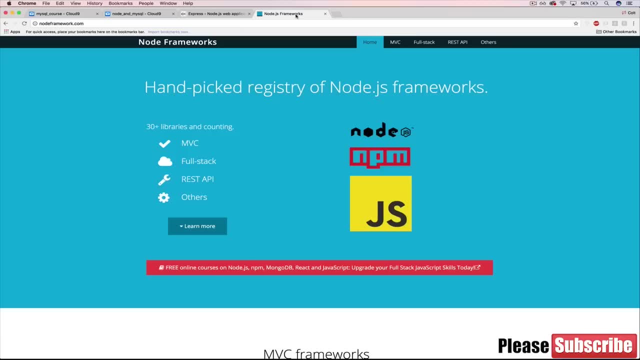 And you can read more about it here. Basically, it provides a robust set of features for web applications. It's lightweight, So what that means. if I go over here to Nodejs frameworks, which is a site that I found, it has a list of some of the most popular Node framework. 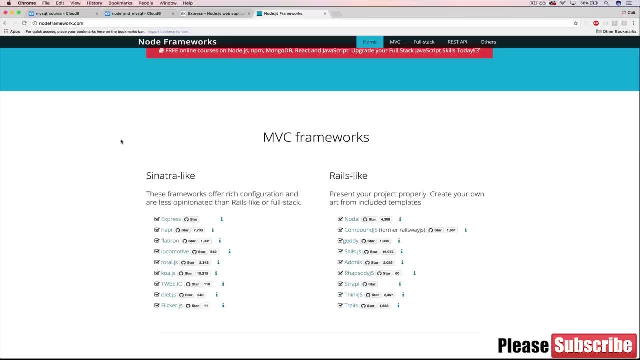 There are a ton of them out there because people love using frameworks, for good reason: They help you make things faster. There's two categories that this person has categorized them into: Sinatra-like and Rails-like. Basically, this comes from Ruby. These are two Ruby frameworks: Sinatra and Rails. 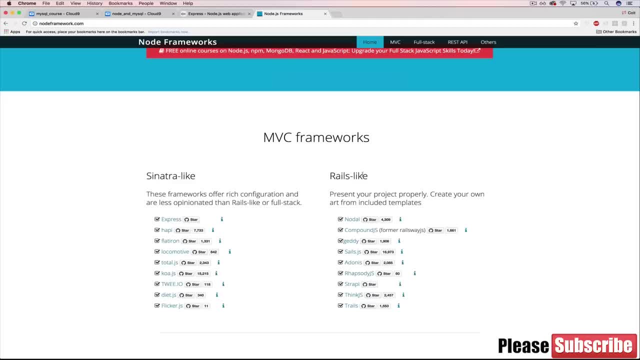 Rails you might have heard of. It's a bigger framework, very popular in Ruby, but it controls everything. It's very strict. Sinatra is much lighter weight, meaning that you have more freedom to make decisions. It's less opinionated, which means that you can configure things how you want. 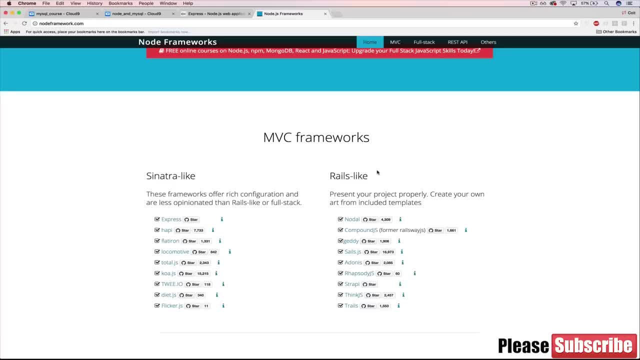 But also the advantage of something like Rails is that you don't have to make decisions, For example, how to structure your files, Where do I put my CSS files? In Rails, you don't have a choice. In Sinatra, you have to decide. 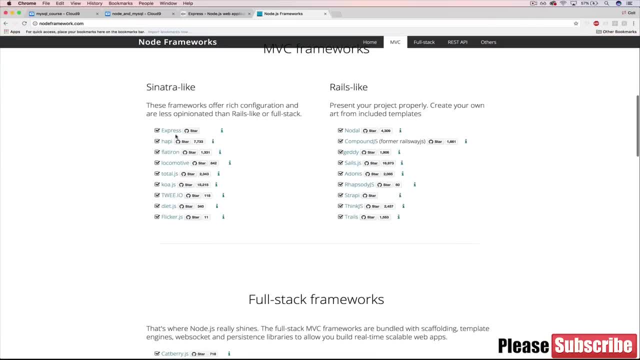 So, with that said, there are all these frameworks for Node Express is the top one here that we're going to use, But there are other ones. There's Sales and Getty are two that I've used. Koa- I don't know if it's pronounced Koa or KOA- is one that's becoming popular now. 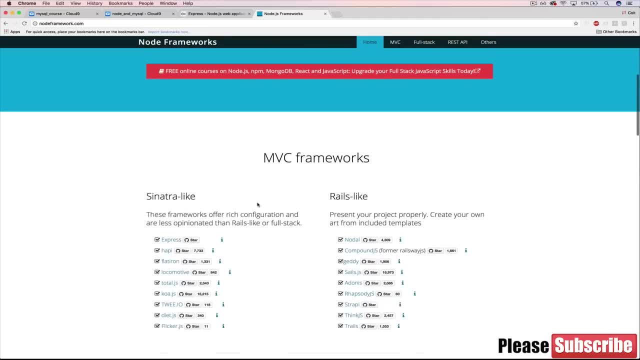 A lot of people are using two. So anyways, I'm just trying to point out here that there are a bunch of frameworks, Just like when I said we could have used any language to talk to MySQL. we could use any Node framework to make a web app. 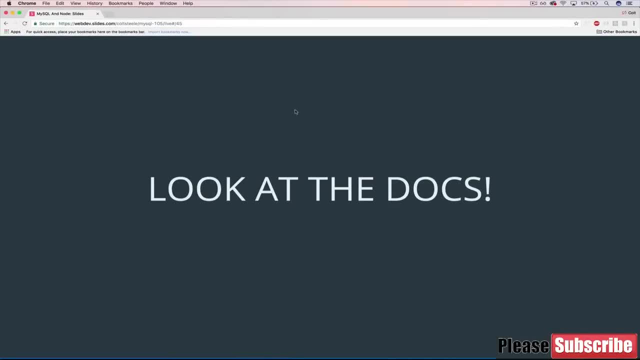 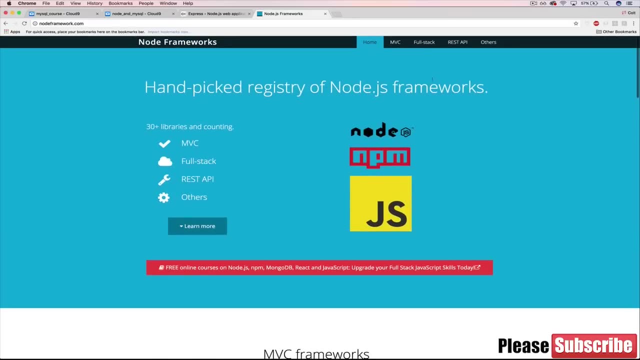 We're happening to use Express, OK. so the first thing I recommend here is to look at the documentation for Express If you're curious, if you haven't taken a course in it, you're not familiar with it or you have never worked with a web framework. 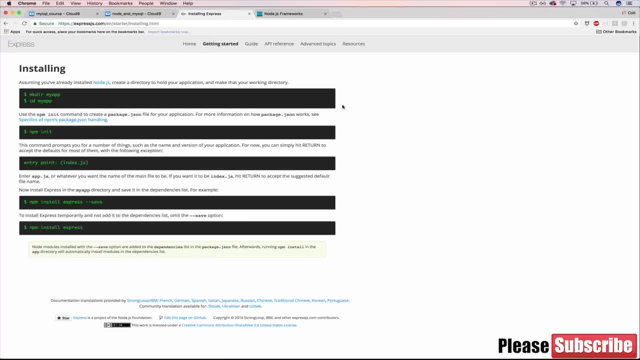 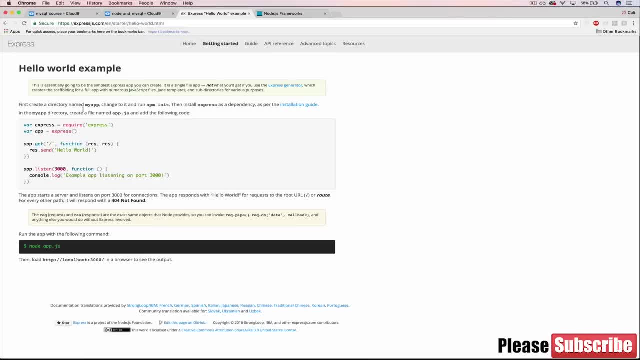 The documentation is pretty straightforward. If you click on getting started, you don't have to go through all of it. But if we actually go to do like a hello world, Here's a simple app that we'll be making in just a moment. 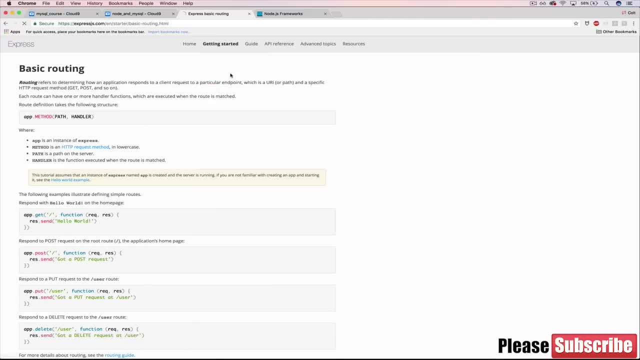 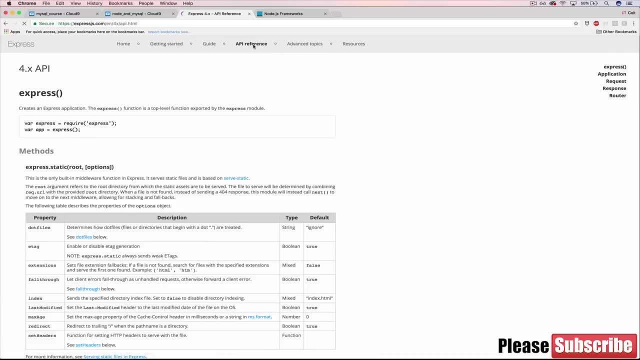 But it has a nice kind of walkthrough of using Express- how you write certain things with the syntaxes- And then there's a guide that's much more in depth And then there's a reference. When you click on API reference, make sure you're doing 4.X, the most recent. 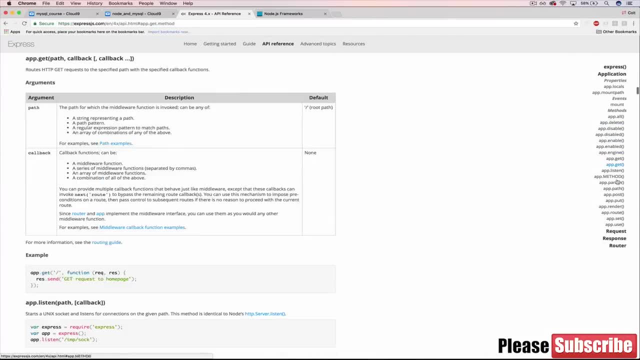 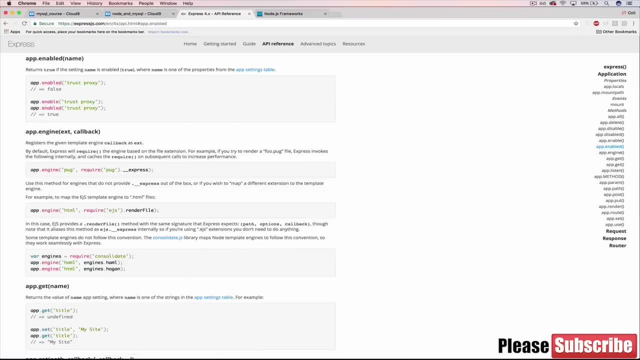 And this is sort of like the think QL docs. there's all these methods that we see over here And you can read about them over here. So we'll be referring back to these docs as we go through the course And for now that's where we'll leave off. 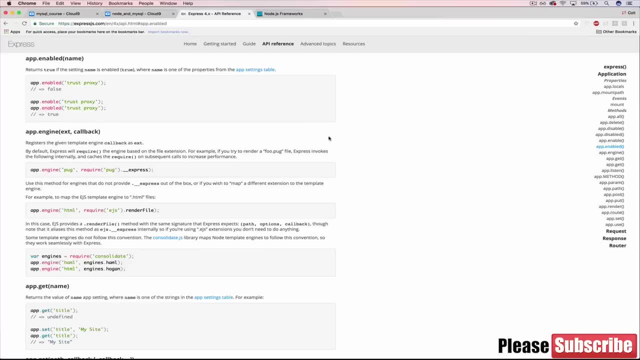 All I wanted to do in this video was introduce Express, tell you that it's a Node framework, show you the website, the documentation. Then in the next video, we're going to install it and create our own first application, First web app. 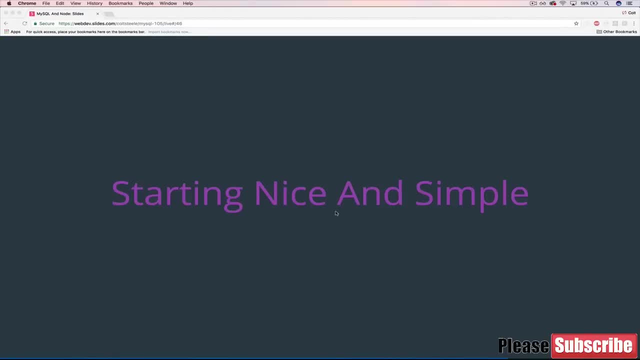 OK, so we saw Express or introduced it. Now let's get down to work, Let's install it And let's make our first simple web app. I don't want to get your hopes up too much. This web app is going to be very, very bare bones. 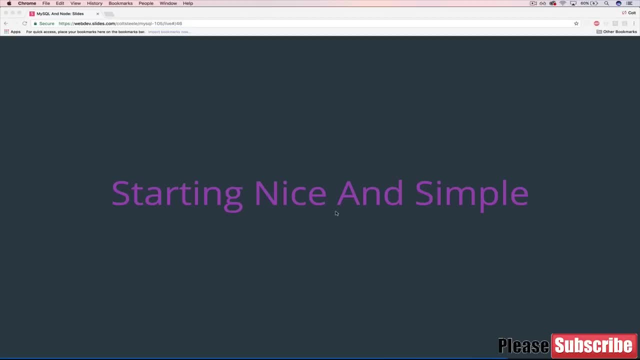 Basically will be a website You hit enter or you go to the URL and we just get a single message back saying whatever we want: congrats or hello or something so nice and simple. But the difference between doing that and then responding with I don't know. 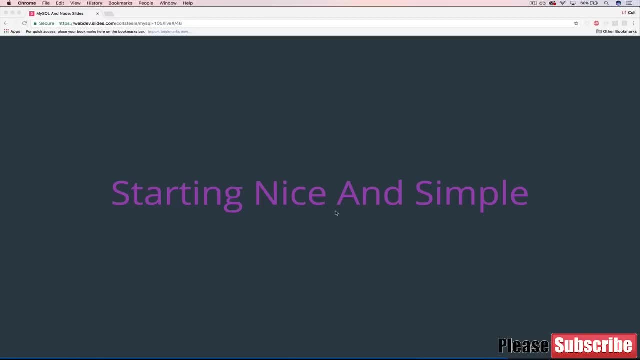 a big, beautiful website with images and big text animations isn't that much As far as the code we have to write on the back, Which is what we're focusing on now. It's the same idea. You respond with some, some content. what you respond with. 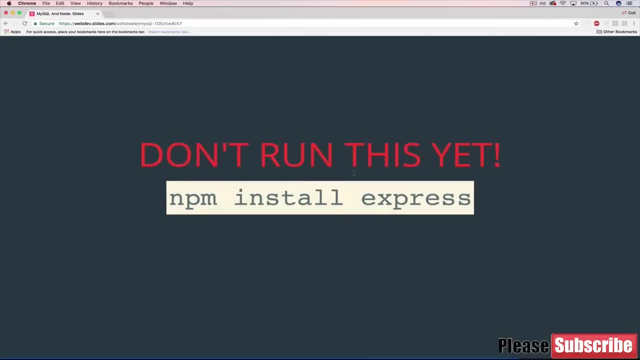 Well, that's a different story. OK, so don't run this. It's a big red letter, say. but to install Express, like we've installed Faker or we installed the MySQL package, you just run NPM install and then the name of the package. 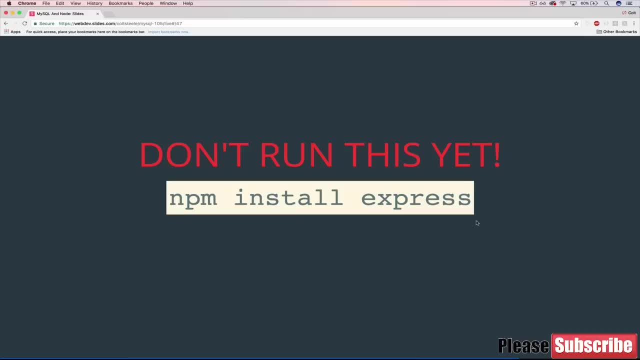 However, rather than doing this, this will work. fine, It will install. I'm going to show you another way of using NPM. That's a little bit nicer, a better practice, And it involves running this first command. What does this do? 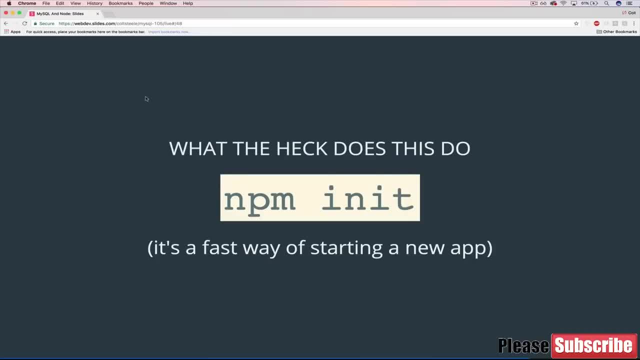 NPM init creates what's known as a package dot JSON file. So if that doesn't make any sense to you, don't worry. Basically, when we make a new project, let's say we're working on a big node project with like a Web app and our Web. 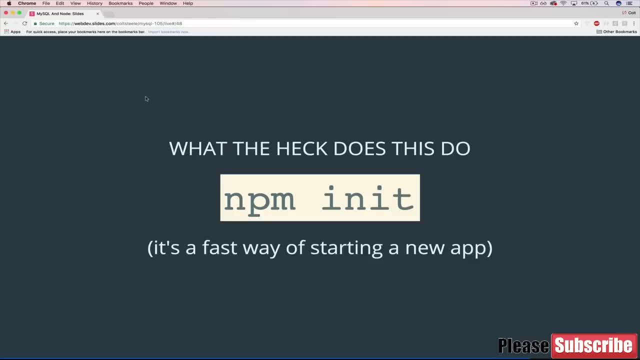 app might have 20 packages involved, so we're only working with a couple right now, but it could have 20 involved. rather than just installing them individually and leaving no record of what's been installed and what version's been installed, What we can do is create a package dot JSON file and it acts as like a log file. 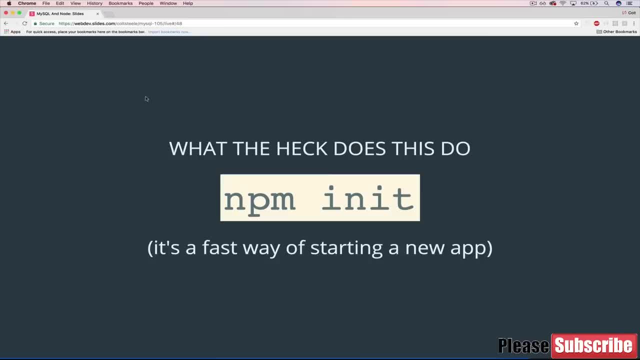 of everything we install, so that if I send my code to someone else across the world or post it on GitHub, for example, all that the person has to do to run it is take that package dot JSON and then run a single command, NPM install. 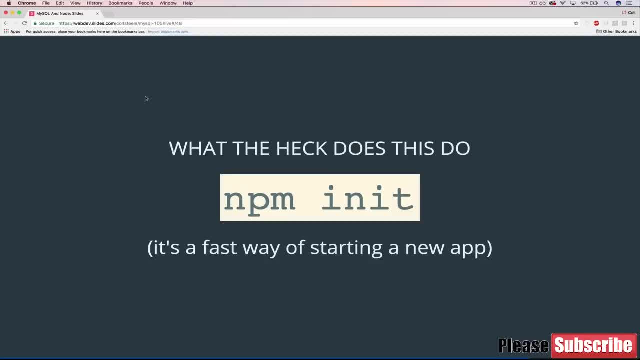 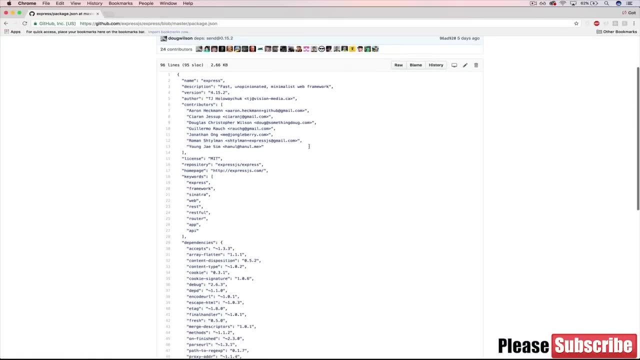 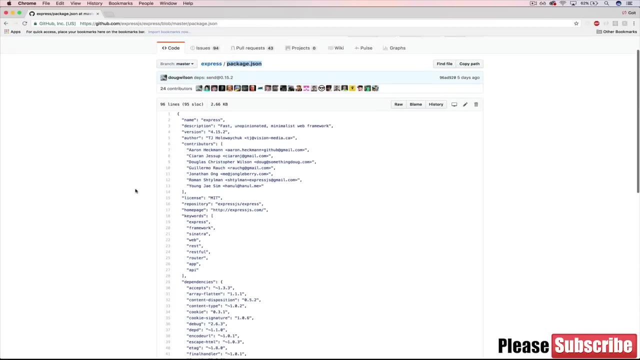 which will then go find the package dot JSON and install every necessary package. So let me show you an example. This is actually the GitHub repo for ExpressJS, the framework we're about to install, which is itself. it's a node package and there's a package dot JSON file in it. 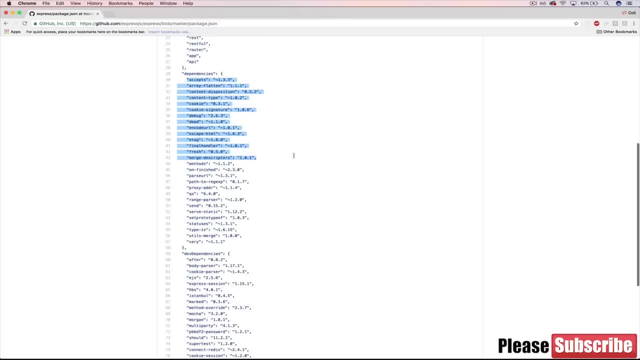 And if you look, there's this giant dependency section. These are all different packages that Express needs. So when we install Express, it goes and installs all of these things as well. So we don't have to do it right If this package dot JSON wasn't here. 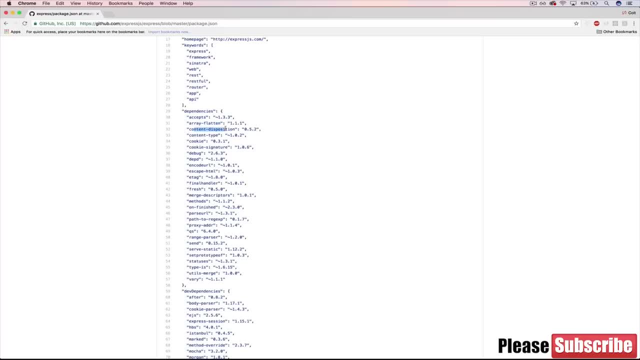 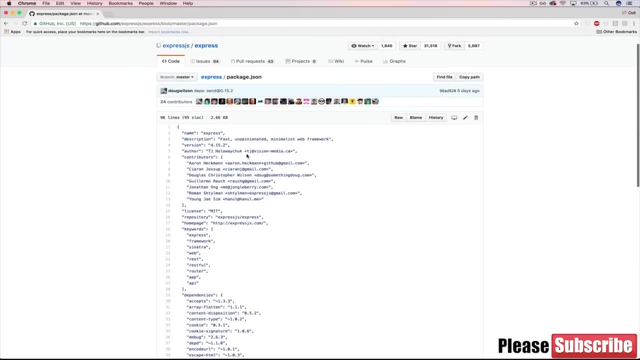 we would have to manually install array, flatten and content disposition cookie. Thankfully, we don't even have to worry about what these do, let alone the fact that they exist. So that's the point of a package dot JSON: It's a way of storing not only the packages that are necessary. 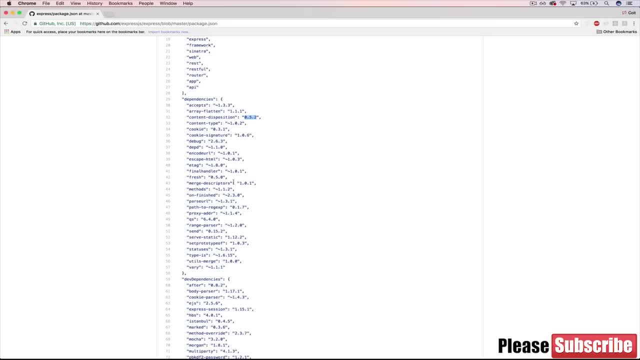 but then the version, because this version of Express might be totally broken if we used zero point six. if that exists, or escape HTML: zero point, zero point three instead of one point zero point three. So that's all we'll say about it for now. 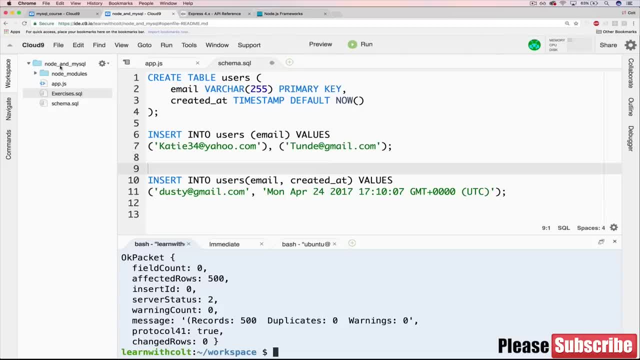 But to actually create the package dot JSON, what I'm going to do is first make a brand new folder, just so that we're working in a different folder, And I'm going to just call this one. join us, And that's where we'll be building the application. 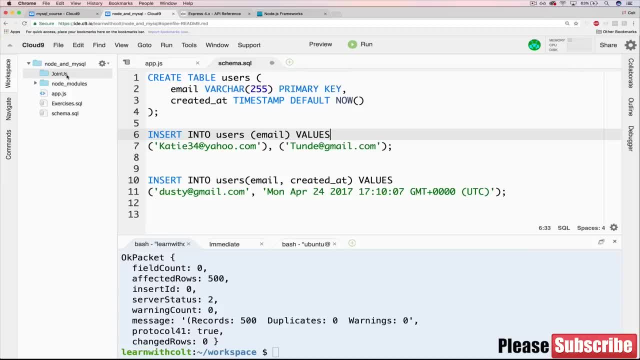 So everything else we've done up until now hasn't actually been building the app. So what I'll do is now CD into join us With the terminal down here, and it should be empty. if I type LS, We're now in this directory. there's nothing there, so we're going to run this. 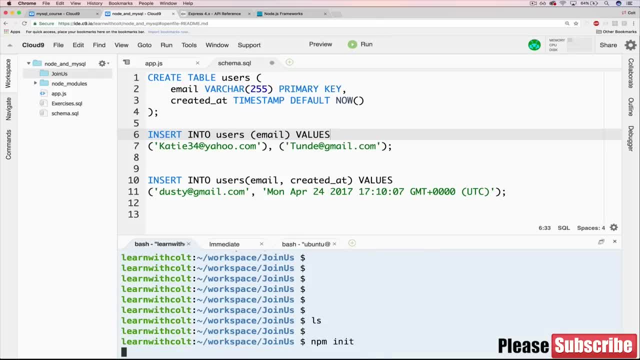 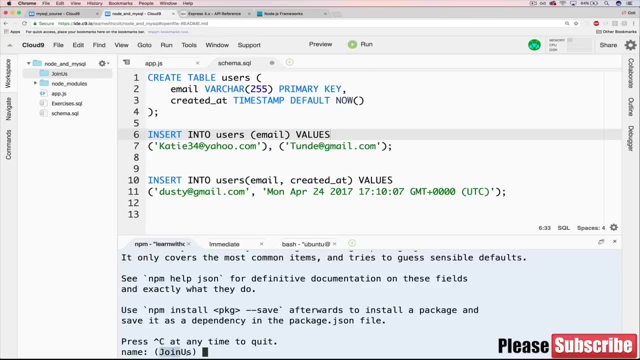 command and this will just generate a new package, dot JSON. However, it's interactive, so it's going to ask us for a name And what you can do is just hit enter if you want it to just accept what it's the default value is. But if I hit enter now, I'll get a message. 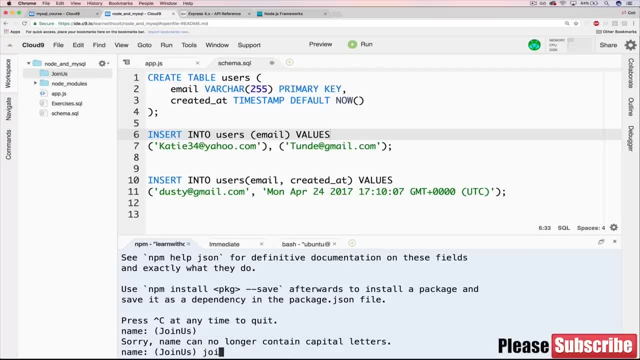 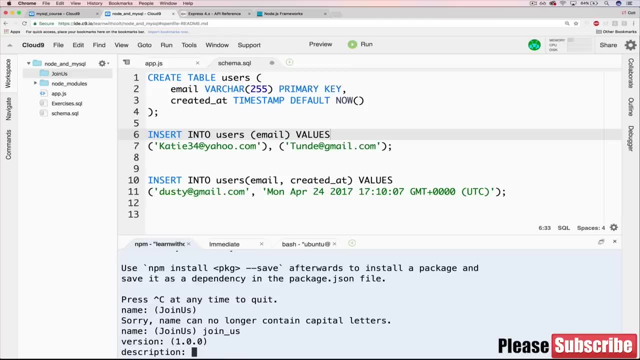 saying sorry. name can no longer contain capital letters, So let's do join us. Underscore version will say: it's one point over app. that's fine description and we can leave it blank for now. entry point I like to change. 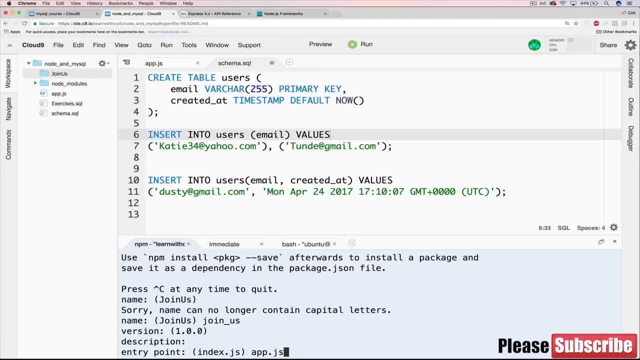 it to app JS. This is just the name of the file that we're writing our app in, or the main file of our app. We could have 20 files, but what's the start point? Index is fine too, but I'm going to do app. 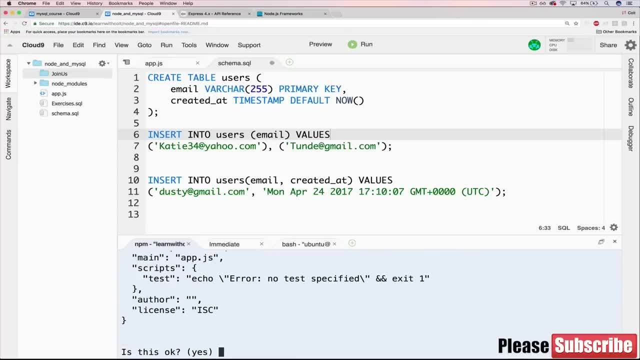 Then I'm just going to hit enter until we're done. You could put author in there as well and a license. Then you can see the, the basic text it generates for us, the JSON, just the data format, And I'll hit enter. 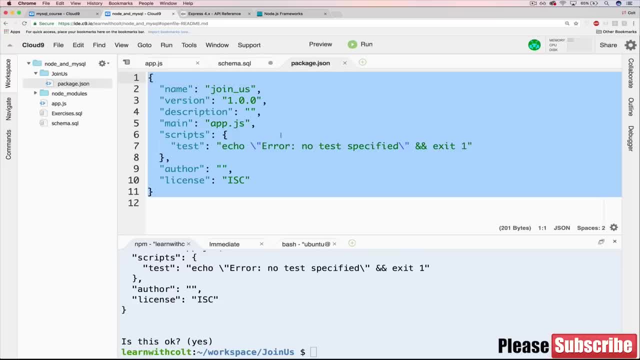 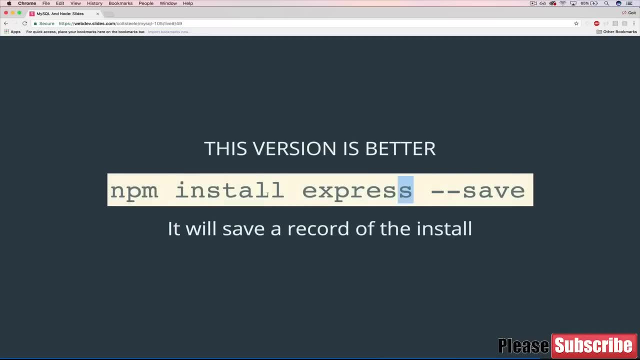 Now I have a package, that JSON file, up here And it's ready for us to install things. So now what I'm going to do is run NPM install express, but not on its own. I'm going to add dash, dash, save and that. 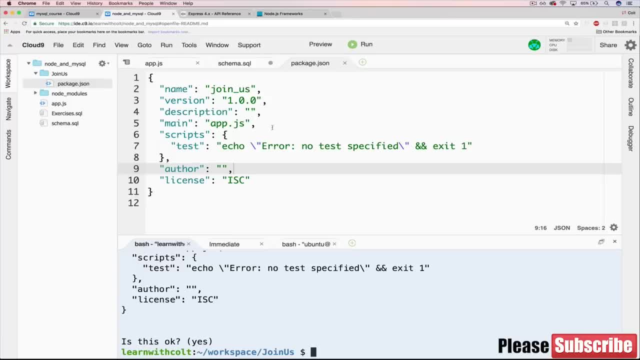 will save a record of our install into our package dot JSON. So right now it's not here, but if I do NPM install express dash dash, save like that Takes a moment, You'll see. first of all, we have our node modules now inside of join us. 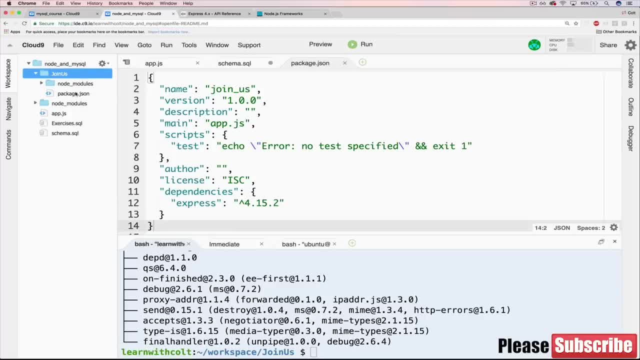 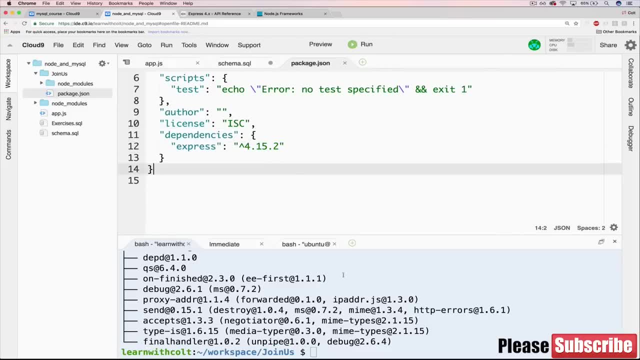 So we installed it in this directory, which is good. Then in our package, Dot JSON, We now have express saying: four point one, five point two is our version. And while we're here, why not also just reinstall NPM? install two other packages we need for our app. 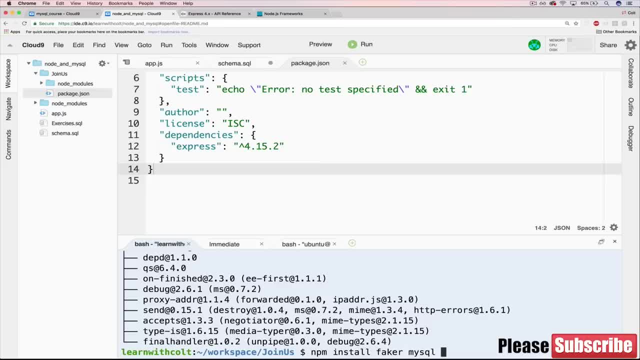 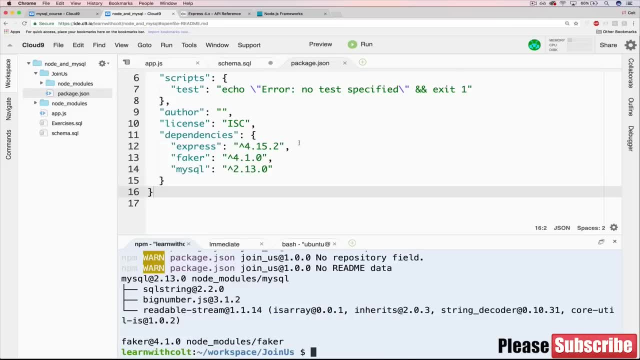 The first one is faker and then the second one is my SQL. You can just separate them by spaces and add dash, dash, save, And then we'll just add both of them in here to not a deal breaker. We already have installed them on this machine, but it's nice. 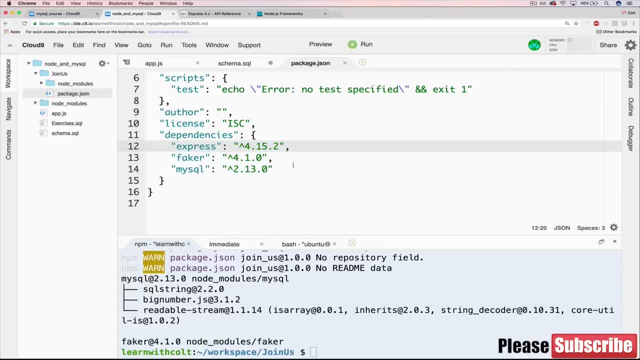 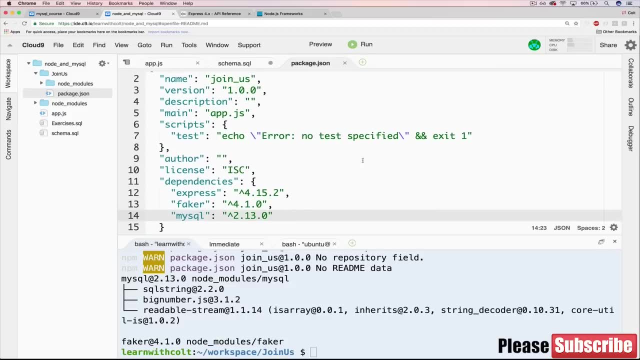 To have them in this directory too and also have records of them in our package dot JSON. So now, if I wanted to upload this to GitHub or something and share this with someone, I wouldn't have to send them the node modules folder and send them the actual express directory and faker in my SQL. 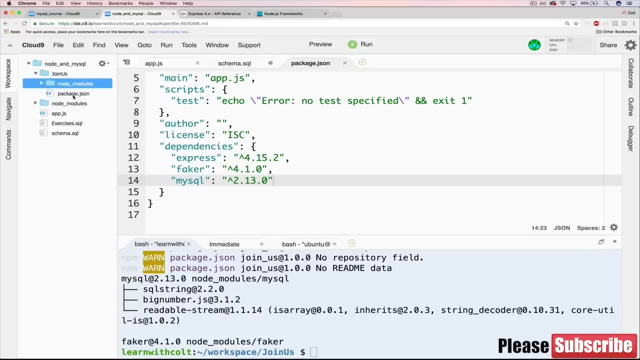 I could ignore that, because this is the largest part of our directory structure Right now. this- I don't know how many megabytes it is, but it's a lot more than this single file or a single app JS file. So it's better to just have our friends. 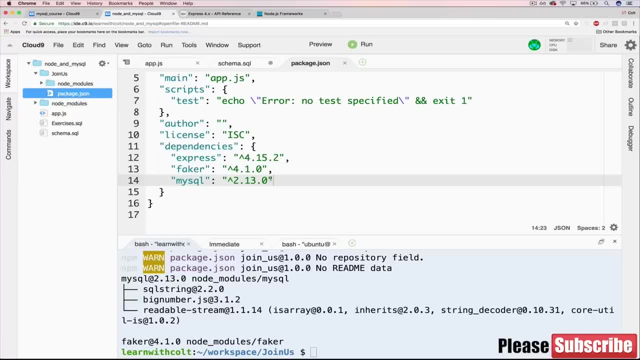 or other developers download what they need remotely. So I just send them this recipe that says: oh, by the way, you need these three things. Here's my code plus the package dot JSON. Then they go, take package dot JSON and they install these things. 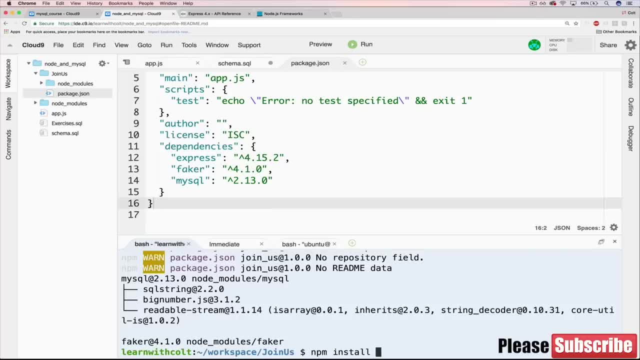 And the way that you do that, by the way, is running NPM install And you don't add anything afterwards. It will try and install everything in the nearest package, dot JSON. All right, So we have express installed. We don't have an app. 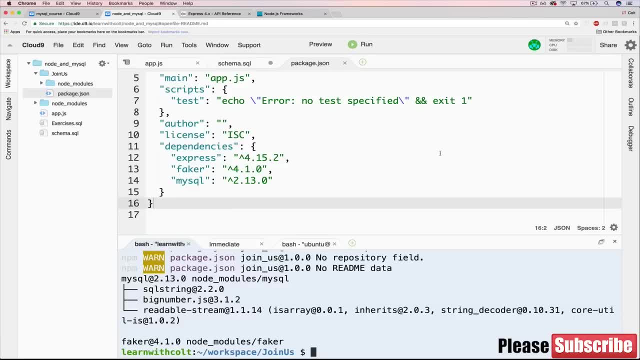 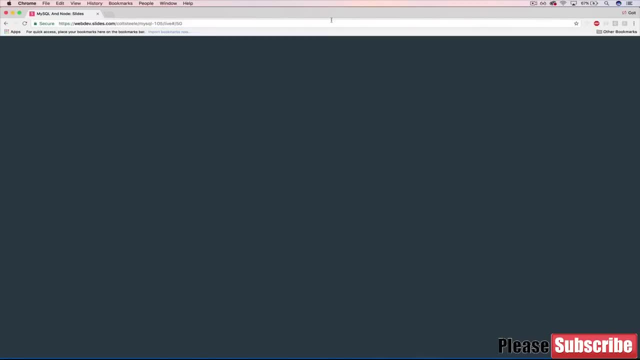 Not yet, Not even an app JS file, But we have the structure that we need to create the app. Well, OK, very enthusiastic. Now we're actually getting to the web app and writing code in this section. In this video, we installed express. 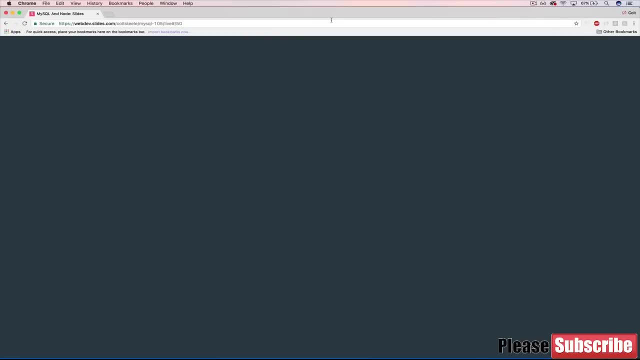 Now we're ready to go, But we need to discuss what we're going to make with our first, most basic pass at a web app. So here's a nice little- hopefully you think it's nice- A little diagram I made of a typical request and response cycle that we'll be working with an express 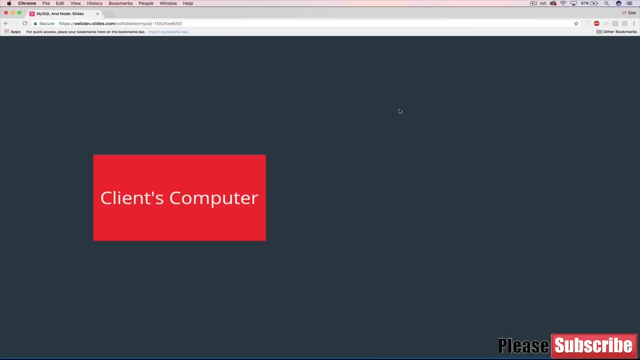 So here's a computer. Let's say: it's blues, my cats. And then there's our express app that we'll be creating, which is node JavaScript and blue types. in the name of our app, Let's just say it's WWW, dot, app, dot com. 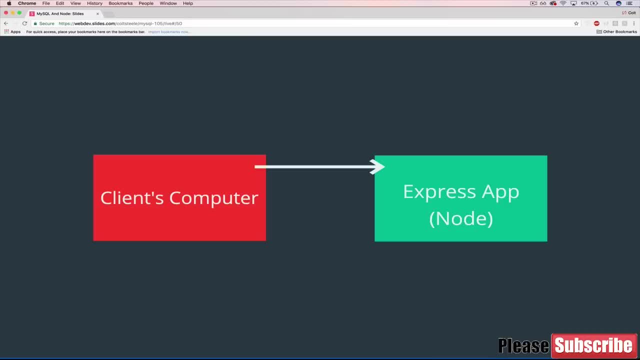 She had center. A request is sent to our express app saying: hey, I would like the slash page, and slash right here is referring to the, the URL that we're asking for the path after. So, if you notice, I'm on web dev dot slides dot com. 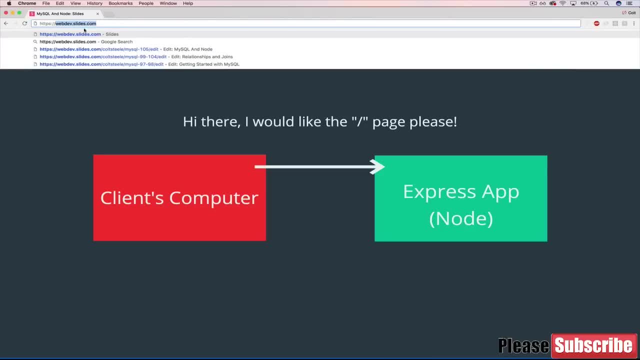 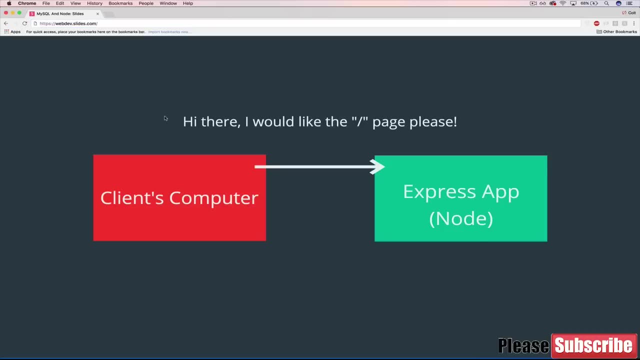 This is basically like our entire express app that we'll be creating, and then individual pages we ask for by varying what comes after the slash. So if you take a look, if you never noticed that before, the path that comes after a slash on a web page, 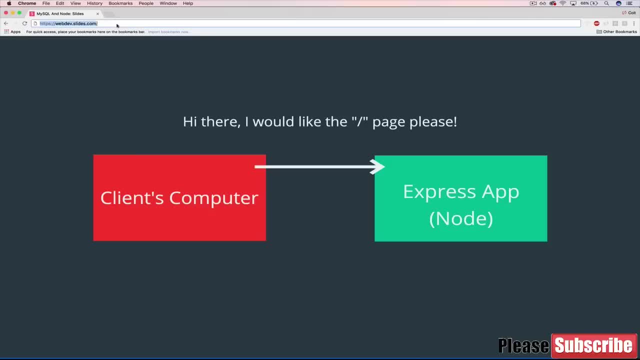 that is usually what dictates what content you see. So when we don't ask for anything, if I just go to web dev dot slides, dot com, that's going to be the home page And the way that we kind of write. that is the path is: slash, just forward, slash nothing. 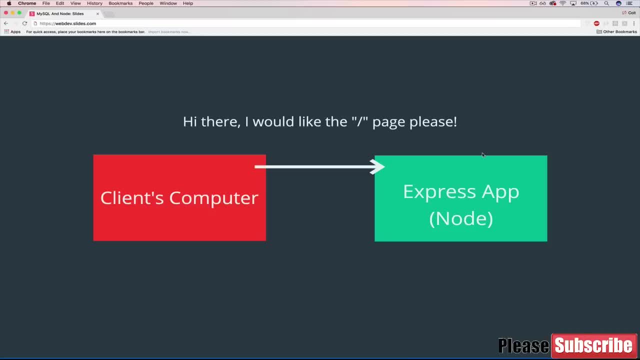 OK, so hi there, I'd like the home page please. And then the express app has to figure out what to do. So it's sure, Here you go And sends back our super simple hello from our Web app. That's it. It just is a one line of text that says hello. 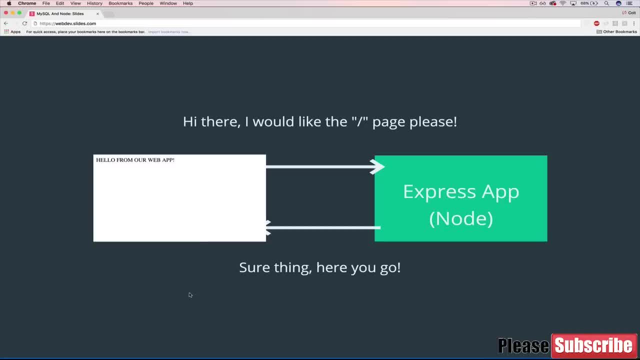 from our Web app. no colors, no animations, nothing like that, And there's no logic involved to start. Every time blue goes to this page, she gets hello from our Web app. Now what we're working towards Is creating dynamic pages that will vary, that will say: hey, we have five hundred. 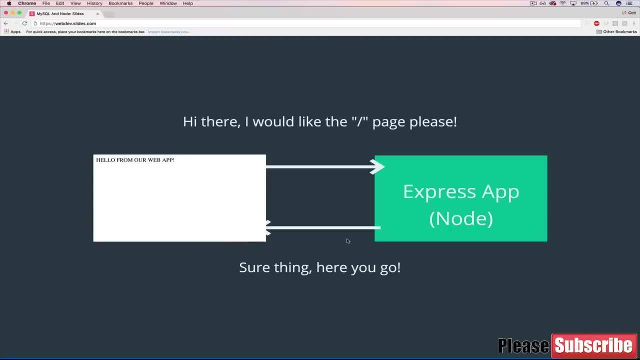 eighteen users, or here's a list of all of our users in the database, or something like that. that varies depending on when the user asked for it, who the user is. There's a whole bunch of different conditions, So that's the flow we're trying to get. 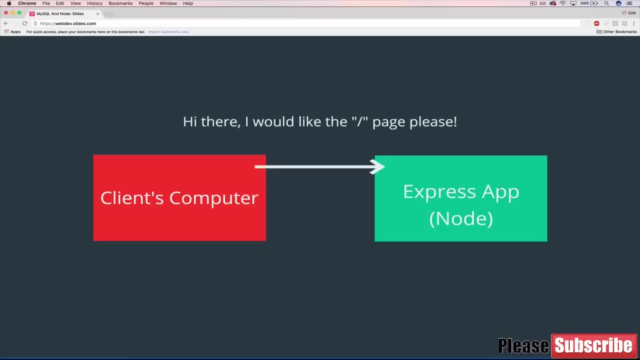 We send a request asking for a particular thing And our express app has to figure out one. how to handle that. How does our express app know what we're asking for? Second of all, how does it respond? So it's these two arrows that are really the important part: the request and the response. 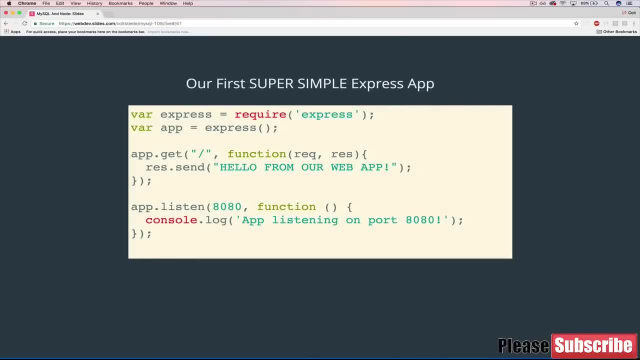 So let's get started. Here's what the code looks like. So there's a little bit here that we have. Well, we haven't seen any of this. we've seen requiring, So all we're doing is importing express and saving it into an express variable. 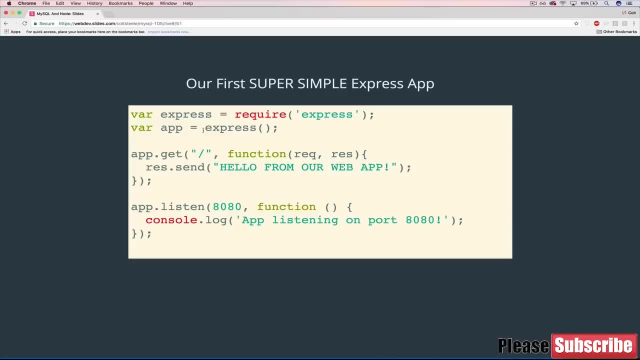 Then we're doing this weird thing that we haven't seen where we're actually executing the entire express package that we just imported and we're saving that to another variable called app. Basically, these are the first two steps of any express application. Copy and paste them every time. 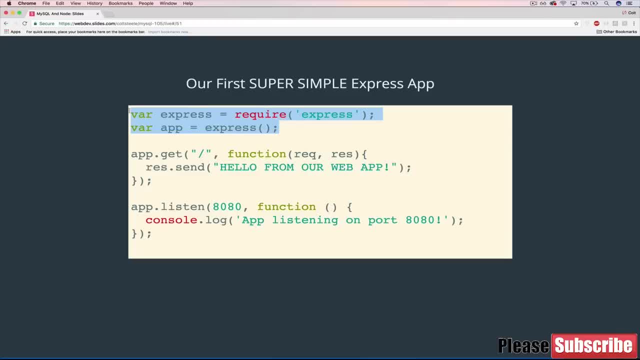 I mean, they're not very long so you could just type it, But you can treat them as just cookie cutter every time. Then every time we refer to this app, like we have here, appget and applisten- both of those are referring to this app. 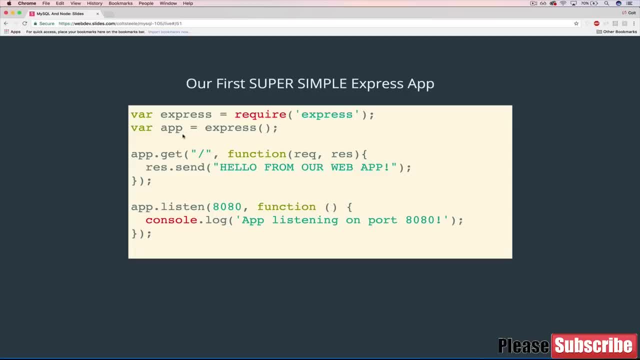 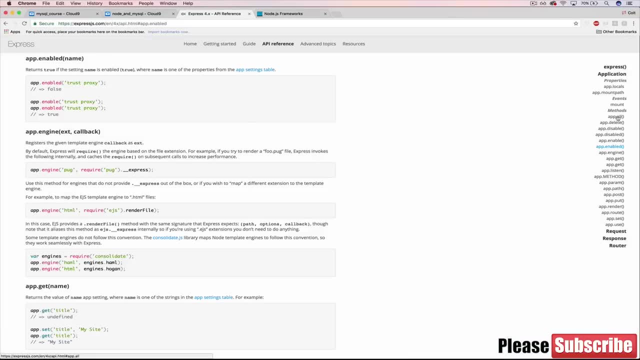 So any time we work with express it's going to be a lot of appsomething, appget, appget, app, All these other things Which on the documentation you can see over here, we have all these appdelete. 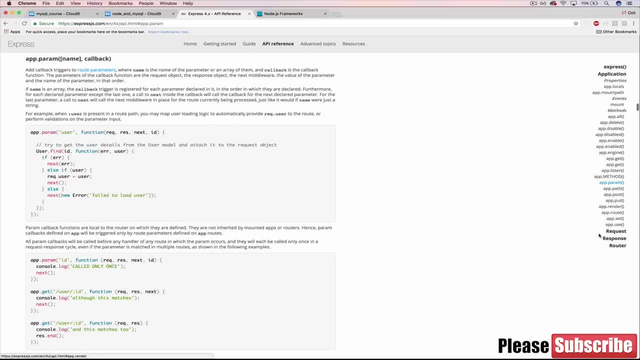 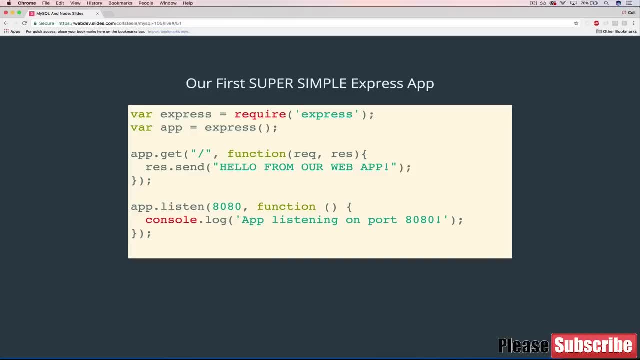 appenable: appget, applisten, appparam, all these different things. They all start with app. Of course, if we name this variable something different- apple- then this would be appleget and applelisten. So so far this doesn't do anything. 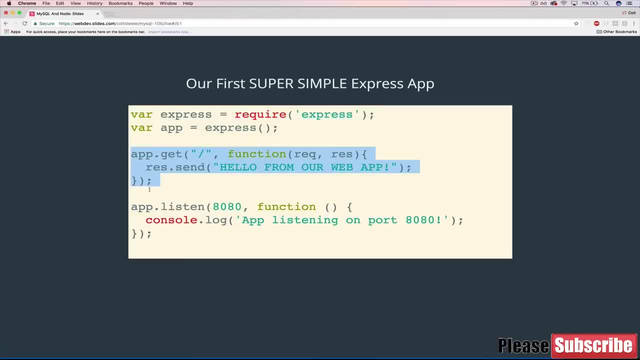 These are just two lines to require stuff. The magic is really here and here. The first thing is what's known as a route. This is the bread and butter of express Every web framework. What it does is this code inside is only triggered whenever a incoming request is made to this path. 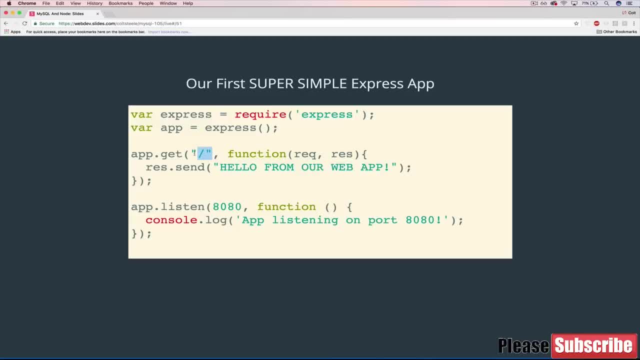 So we're basically defining the code that runs when a user asks for a home page where the path is nothing, It's just slash. And what are we going to do? Well, we are going to send. this is a special method from Express. 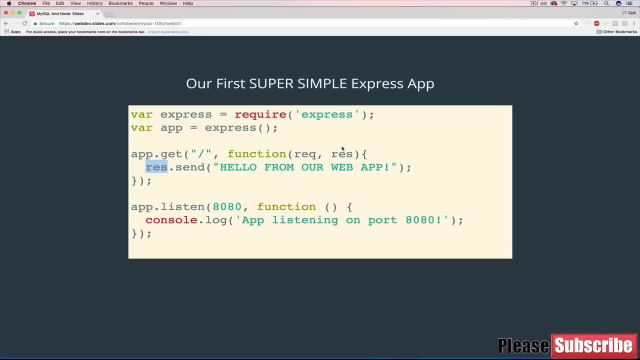 Hello from our web app and res is coming from here. There's a lot to take in. I know res is the response object Request is the incoming request, So every route there is a callback, Just like when we were working with MySQL. 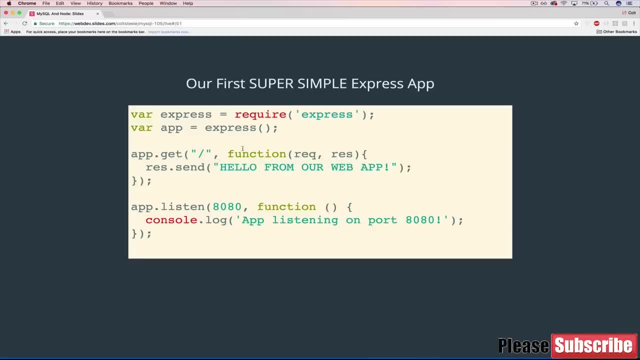 callback is code that runs after something happens or at a later date, So this code only runs whenever a request is hit to slash. So eventually we'll have code where we have five or six routes- different web pages. We want to run different code depending on the web page that's being asked for. 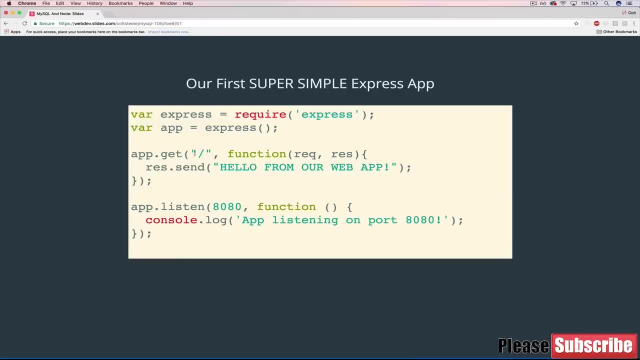 So this is how we do it. This is basically saying: if a request comes in for slash, run this code. We could have another one down here that says: if a request comes in for slash log out or slash log in, then do something else. 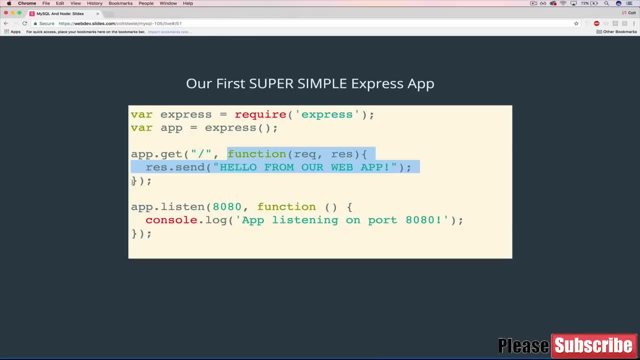 Show the login page. So that's the first bit. Then every route has a function, a callback with two arguments: a request and a response. Request, again, is the incoming request. So if we wanted information from the incoming request from the user, which we'll be working- 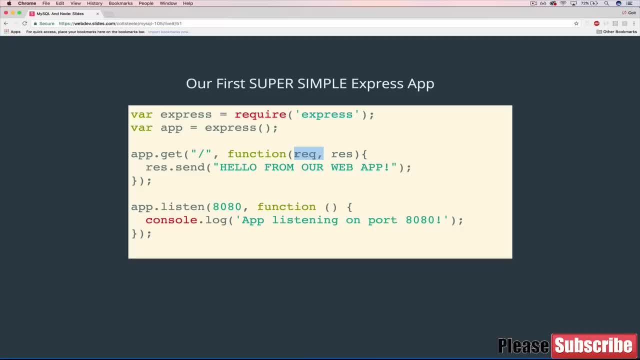 on later. when a user types their email into the form to sign on to our waitlist, that information is sent to us, and so we'll need to work with the request coming from the user. it's this arrow that will contain the information. 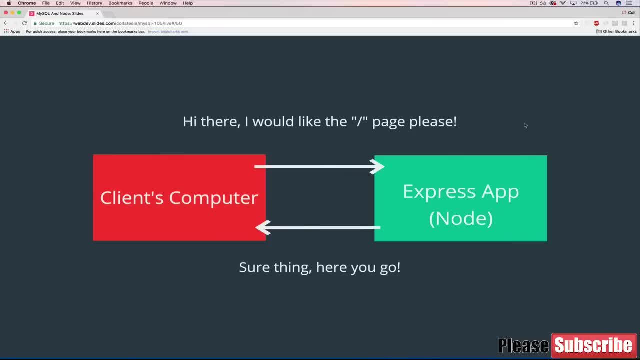 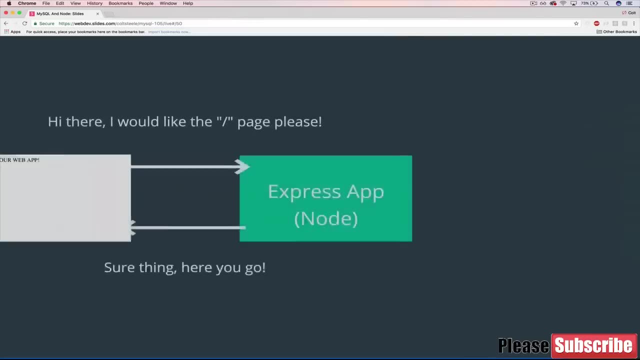 Hello, I'd like to add my email, blue at gmailcom- to your database And so then with the request, we'd be able to pull it out of there. The response is what we're sending back. It's this arrow going that way. 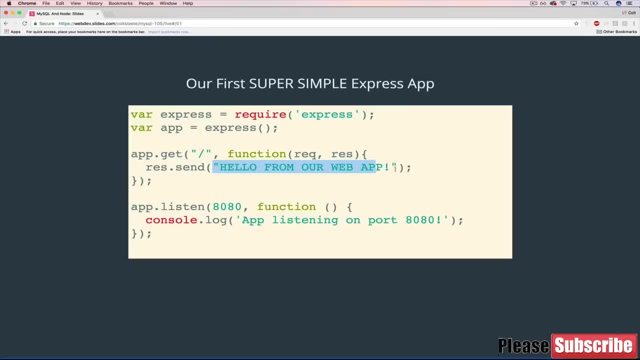 And so that's why Res dot send hello from our web app will send this response. Of course, you don't have to name it rec and res. You could call this request and response. You could call it R1 and R2, apple and orange. 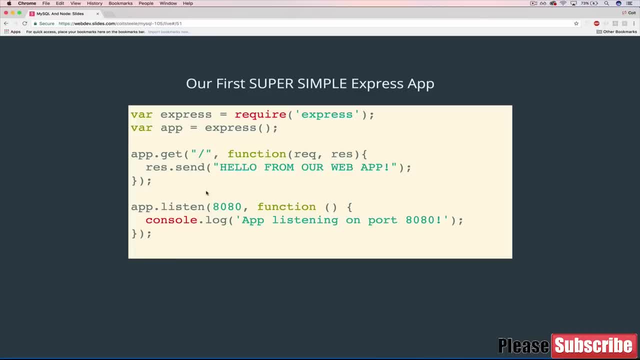 All that matters is that you refer to it the same. And then we have this second component, and this is also kind of cookie cutter. You'll have this in every app. app dot, listen, And all that this does is starts a server. So this starts the server going. 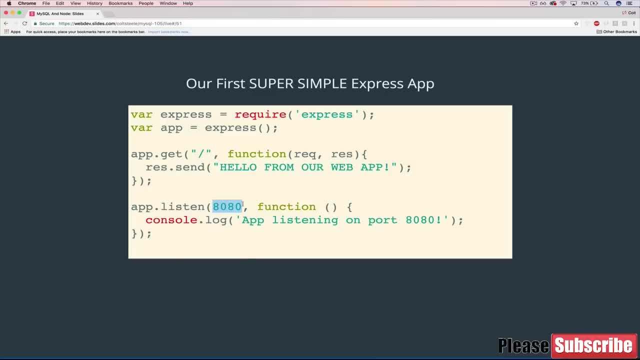 We have to tell it what port which, on cloud nine, will always be using 8080.. And then, if we want, we can give it a callback function. And this is just a line of code that will run once we start our server. 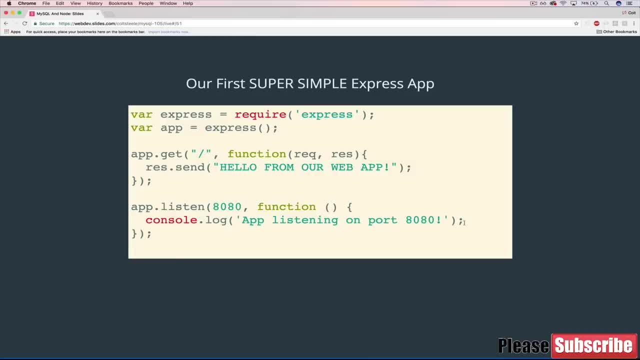 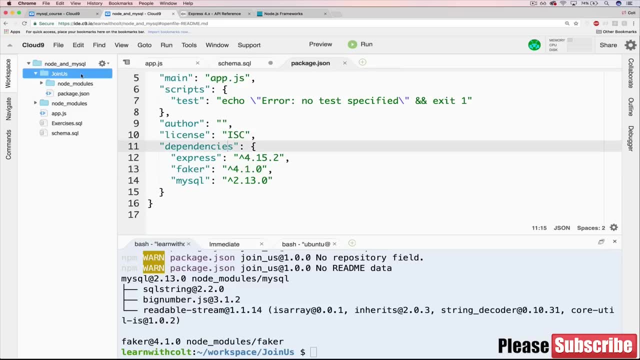 So it will just say in our terminal: hey, your apps listening on port 8080.. You don't have to have this. So let's go over to cloud nine And the first thing I'm going to do is make a new file. 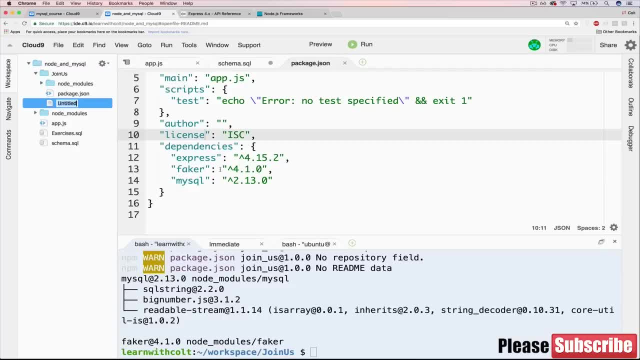 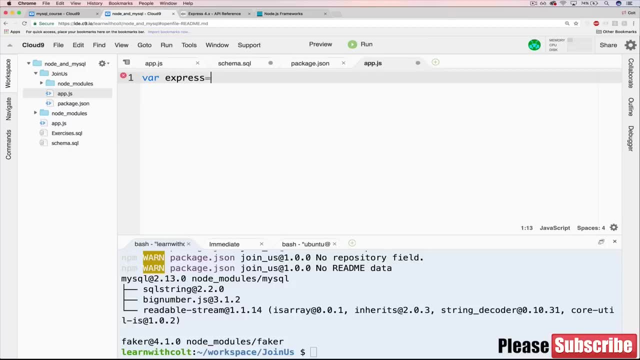 So, inside of join us new file, And it's going to be app dot JS, And I'm going to just start by requiring express, just like we saw. Then I'm going to do our app equals express, which is referring to this executed as a function. 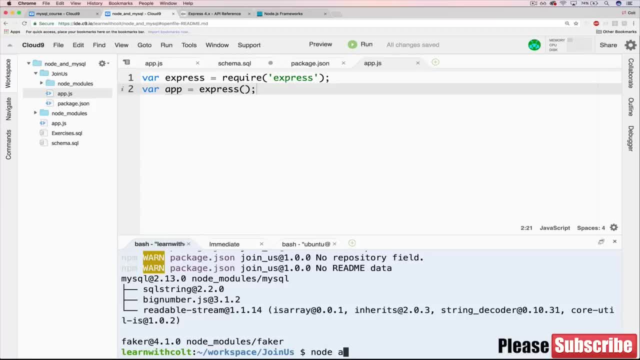 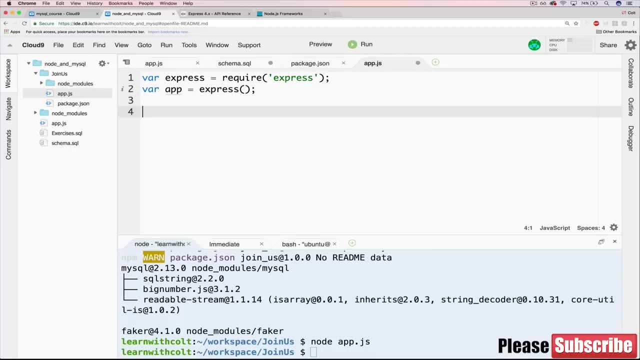 So we have app there. Let's just see if it works. Nothing will happen. We may get an error if we didn't install express, but we did, So everything's good. Then let's start actually at the bottom. So we start with our app: dot listen. 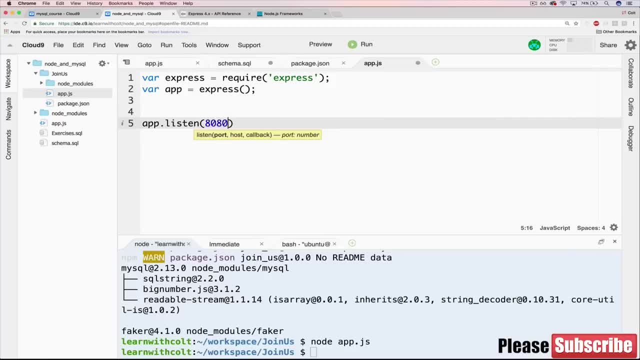 And we tell it the port which is. if you're not familiar with the idea of ports, think of it as the entry or exit point on a computer. You can have 20,, 50, 100 different ports for different things going on at the same. 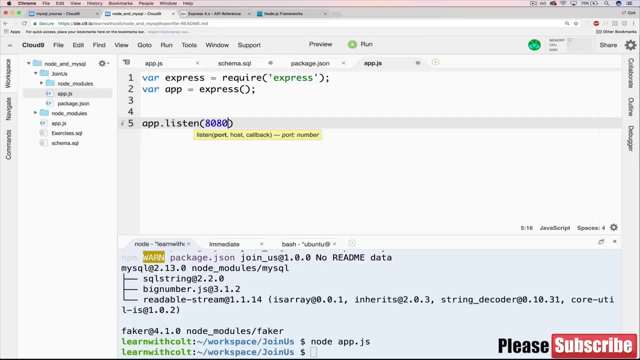 time You may have had to work with ports, if you ever had to like mess with a firewall that was blocking something you didn't want it to block, Or if you work at an office where they- I don't know they- don't allow you to go to certain websites. 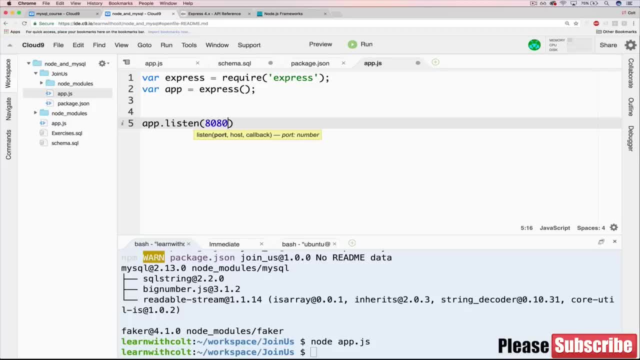 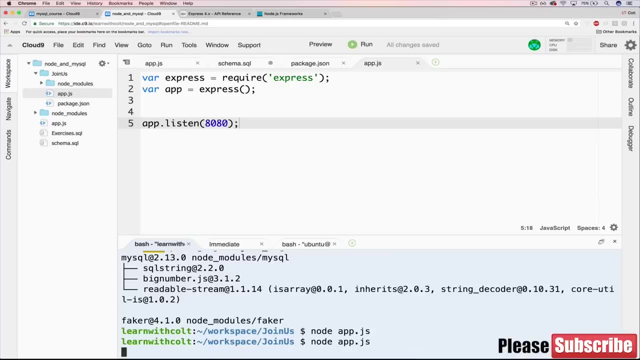 That's running on a certain port. Anyways, app dot listen 8080.. And we could just leave it at that like this. But if we do that and I start it up, notice my cursor has gone to the same thing that happened with the MySQL connection, when we didn't end the connection. 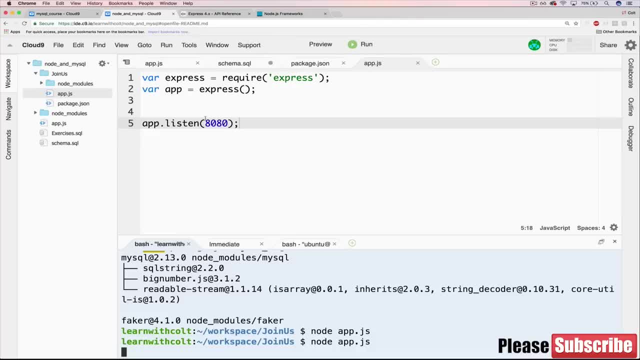 It's just hanging And that's because I started the server. It's listening on port 8080 to see any incoming requests, But we're not doing anything And it's also just not very. you know, it's not a great experience to just see a blank cursor there. 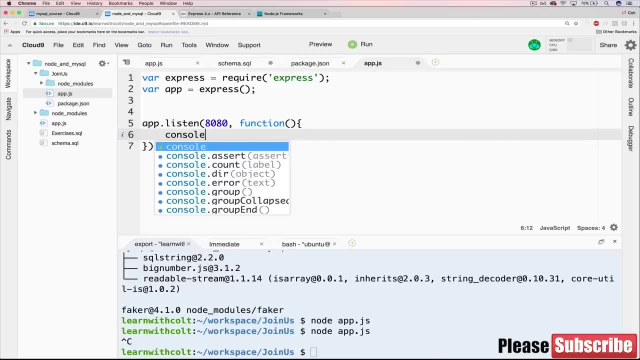 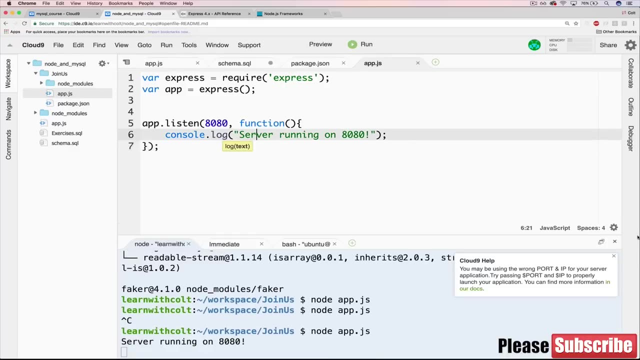 So we can just add this blank callback And it will just console dot log server running on 8080.. And it's just a nice message for us developers to see. So now, if I do it, you can see, of course, that we get console dot log server running on 8080. 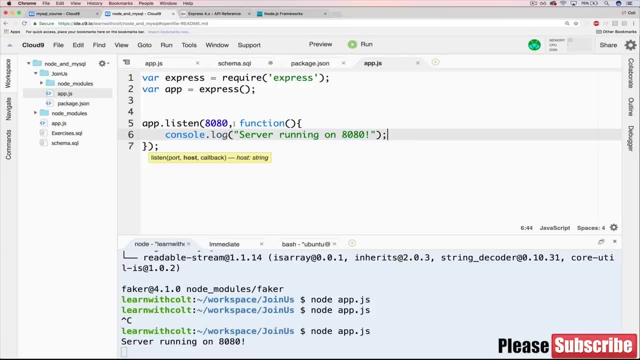 And that's just because this code runs. whatever we put in here will run only once the server starts. So that's the first thing. But now we have the task of actually writing the code. So we have our server, It's going, But we can't actually reach it. 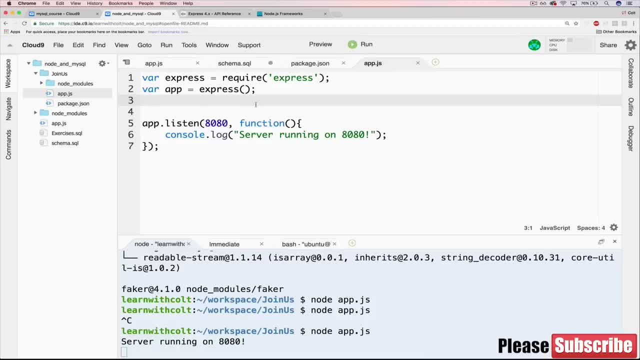 We can't do anything with it. I don't have anything to respond with. So actually what I just said is kind of a lie. We can reach it, We could request it, but nothing would ever come back. And actually, if I try and preview it right now, 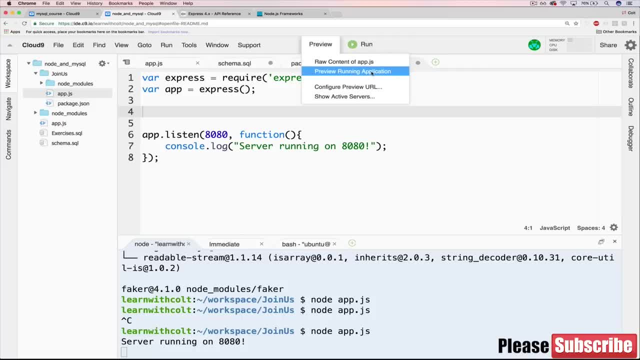 So to do that, we can click on preview. preview running application. This is hitting this server, but we're not getting any response, So I'm going to just leave it here for now. We'll come back to that. We'll know that our app is working if we 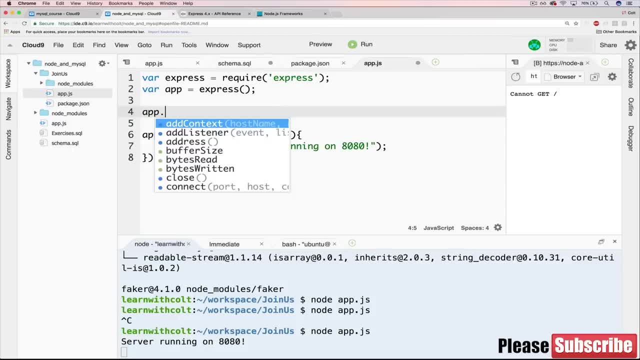 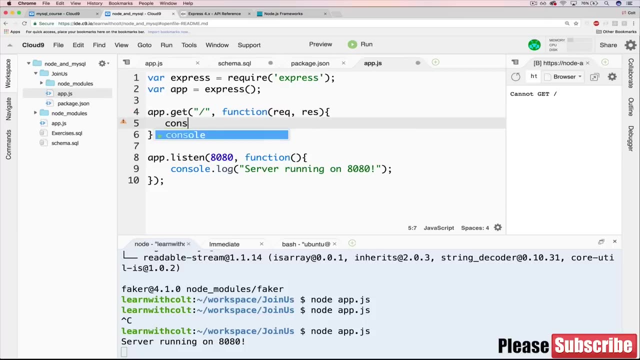 get a response here. To do that we just have to do our app dot get And then you are the path which is slash function request response And then in here we put some code so we could start with just a console dot log. 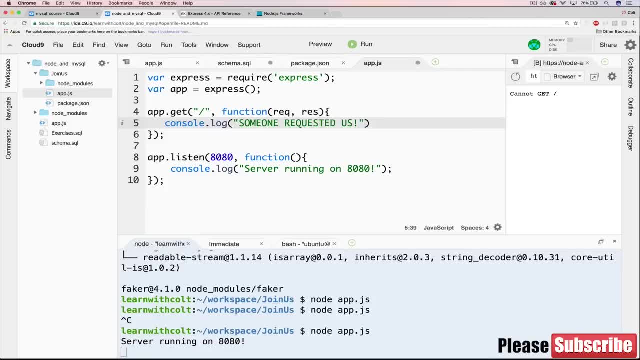 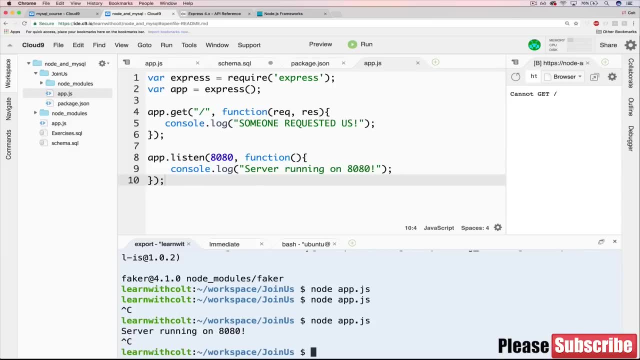 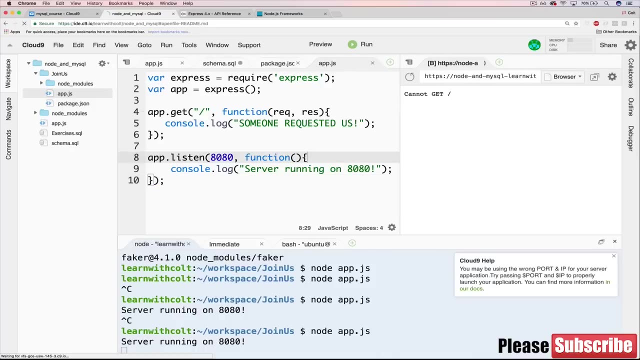 Someone requested us just like that. What do you think will happen? First thing you have to do is restart the server any time you change this code in here. The server was already running. We need to save the file and restart. But now, if I try and request slash, I'll just hit enter here. 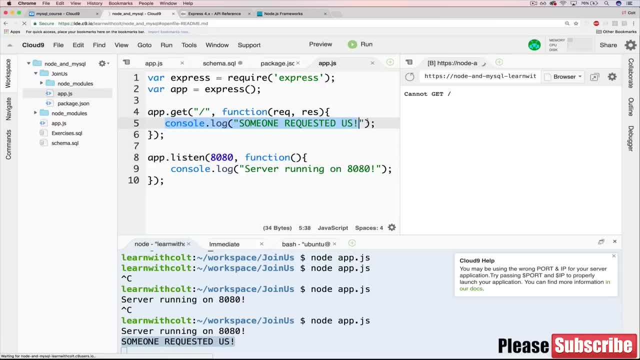 Notice what happens says someone requested us because this code ran, But over here we still don't see anything. So console dot log is only printing to the console, here the terminal. So now what I'm going to do is open a new tab and put this in that tab so that we have our app and then our terminal. 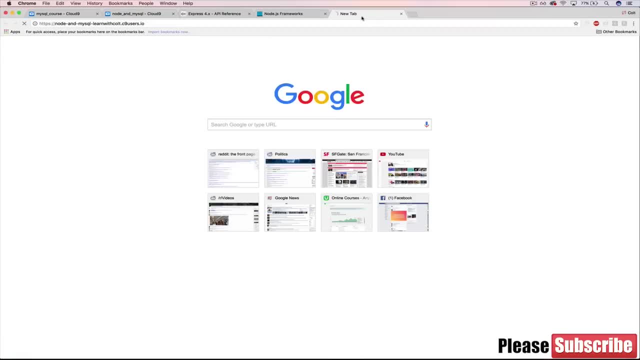 Down here, and I'm going to close this one just to make more space. It's the same thing. Notice, though, every time I hit enter, I get someone requested us, But if I tried to go to slash, log out or something that doesn't exist, 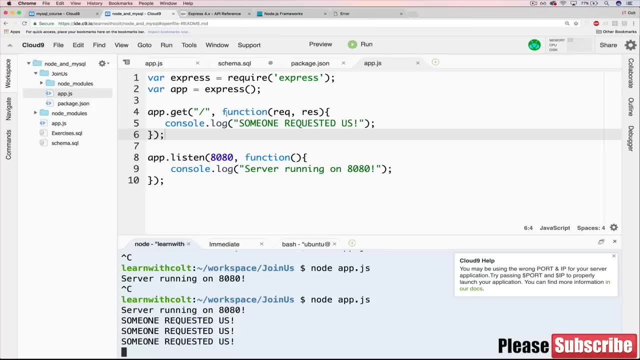 I don't get someone requested us because that this code is only happening. It's only firing off when we're requesting a slash. And you might be wondering about the get part If you're not familiar with HTTP requests. there's a couple of different types. 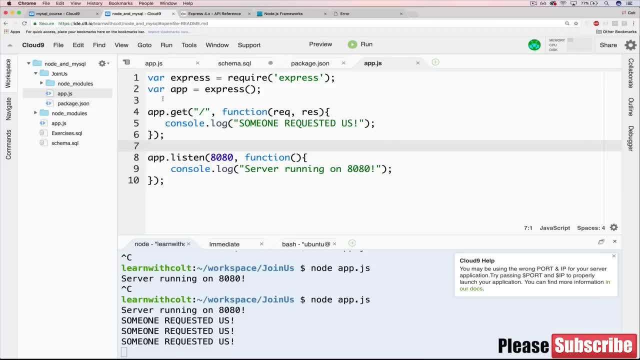 different verbs- get and post- are what we'll be working with. For us, though, think of it as just asking to see information. You're not sending any data with it, So when we are asking for our home page of join us, we're just trying to see information to get request. 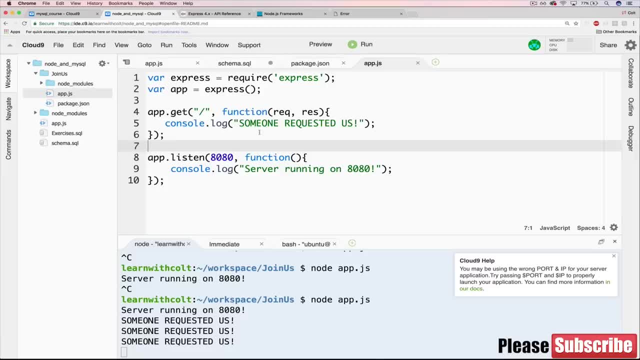 But when we are trying to join we are sending an email and that is going to be a post request. We'll get there in a little bit. I know it's a lot of stuff and overwhelming if you've never done web development, so hopefully you understand. this is not a web dev course. 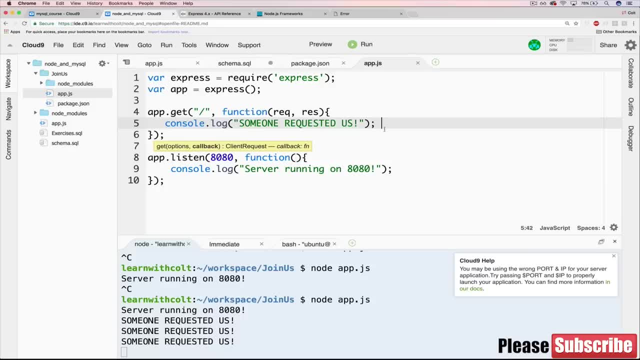 but there are some great ones out there and I highly recommend, if you're curious and you are enjoying this part, that you continue down that path. OK, enough of that. So, rather than just console dot log, there's this other thing we can do. 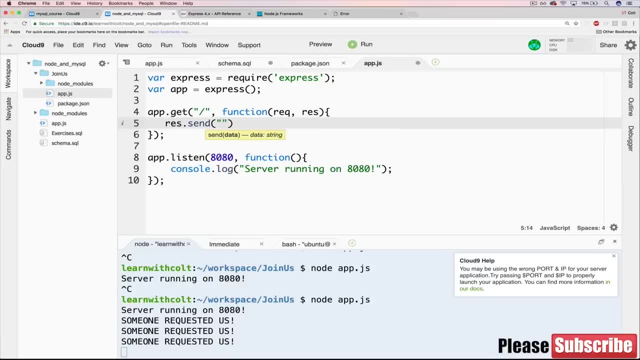 which is response, dot, send, and then we can put any string in here, like you've reached the home page. I'm sorry about that, siren. It's like 100 degrees in San Francisco today. That's a lie, It's 90 degrees. 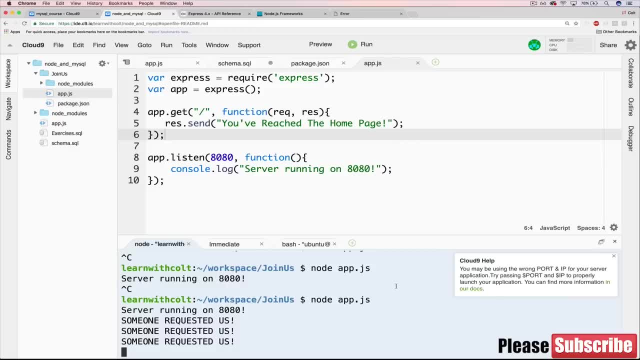 I have to have the window open. OK, hopefully it's not too loud. Now we need to restart the server. This time we now have some different code. Same thing if we hit slash on this app that is running on 8080,. 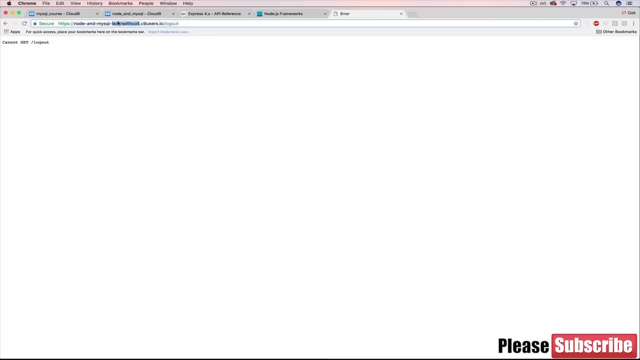 which in cloud nine. this is our URL. yours will be different. You have a unique URL you need to access, but this is where your app will be running, Just like when we first installed Node and I showed you that chat app. It's the same idea. 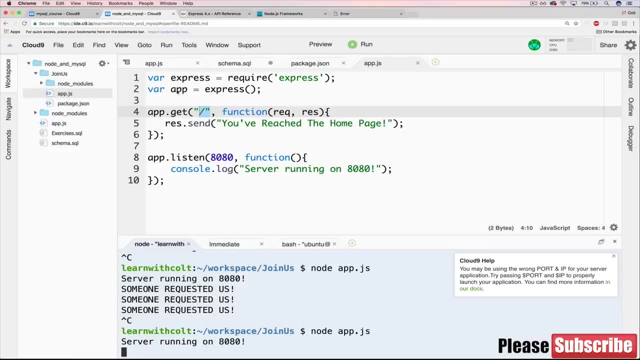 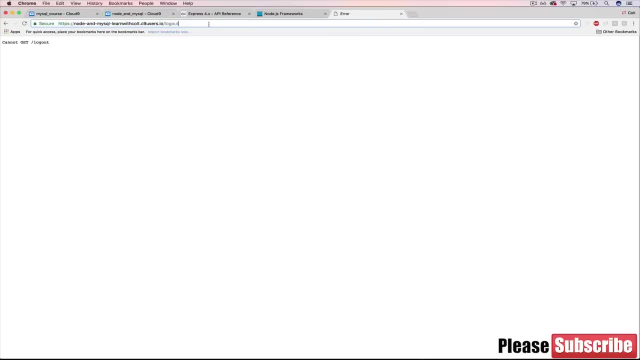 This is where your app runs by default. So now all we need to do is hit that page, but we need to ask for slash rather than slash log out. If I do slash log out, again I get nothing. So if I just do slash or nothing, 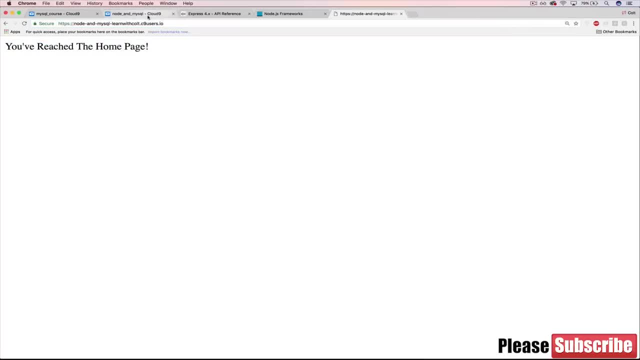 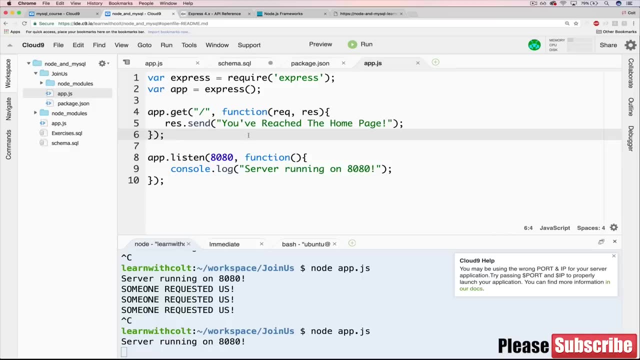 we get our message, You've reached the home page, And that is our most basic Web app. Of course, you could change this text. Something that people ask a lot is: can you have two res dot sends? The answer is no, you can only have one. 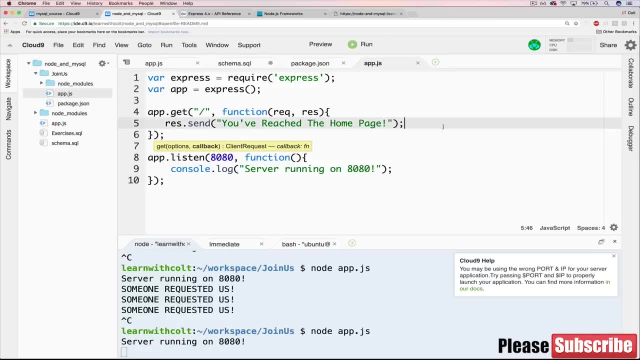 Every route is going to respond with one thing, But the real answer is that you're usually not going to use res dot send. you'll instead be responding with files. So we'll have a file of HTML to respond with our nice formatted page with style and fonts and colors. For now, this is a very basics. 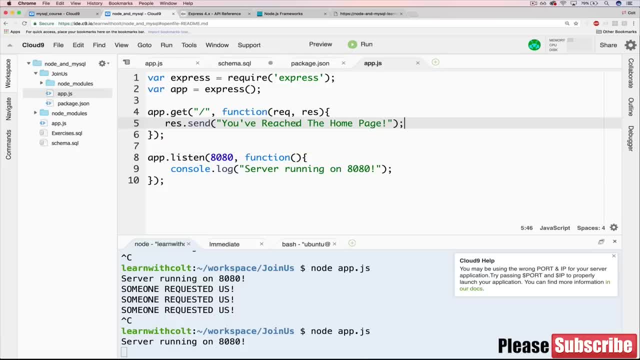 So we'll stop here. You can feel free to move on to the next video where we add more routes, But at the very end I'll take some time to review, if anyone is curious or anyone feels like you need more review of how this works. So we started by requiring Express, which is the library of the framework. 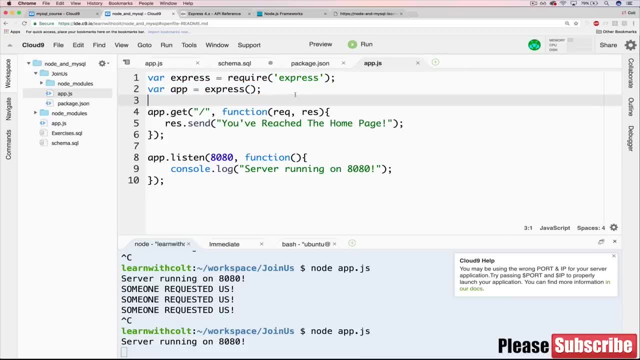 that we installed, Then we execute it and save it to our app variable And really there's a lot of magic happening there. That's what a framework does. It takes care of stuff in the background. But now what we've done is, first things first. 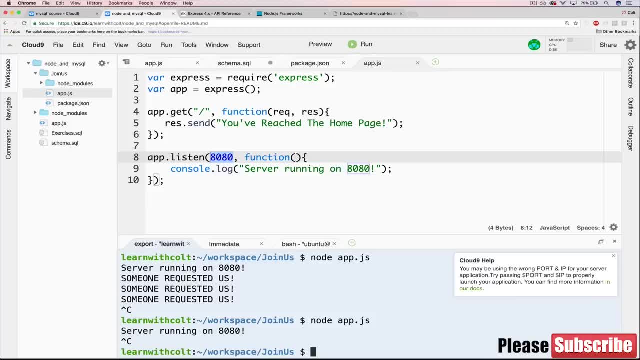 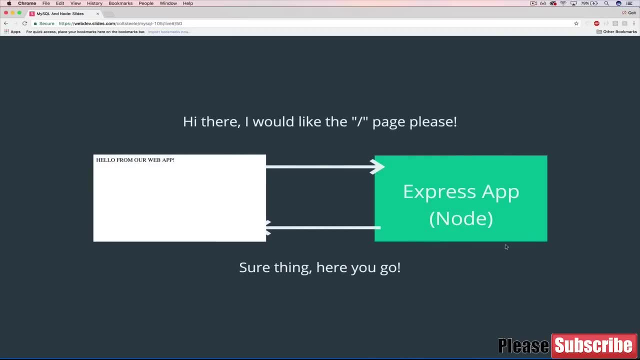 We started up our server app, dot listen 8080.. And every time we do that, our server starts running And basically, that is this block right here represented by this block, And it's just sitting here listening to patient server. Nobody might talk to it. 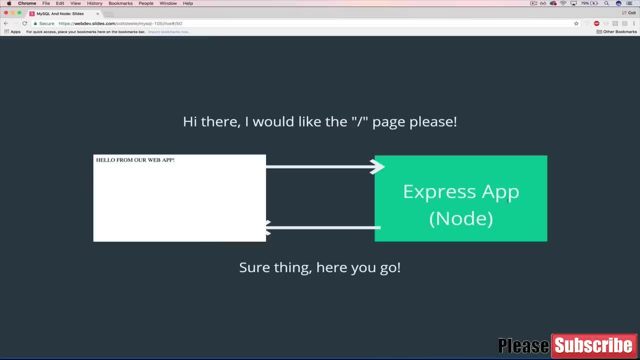 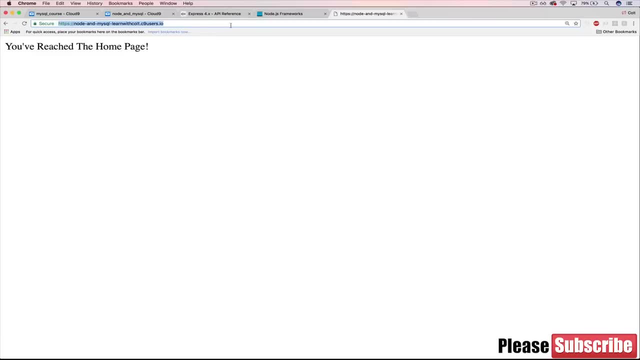 For years or maybe ever, But as soon as someone sends a request and in our case the request goes to this URL node in my SQL learn with Colt dot C, nine users that I owe. yours will be different, But this is where I make a request to. 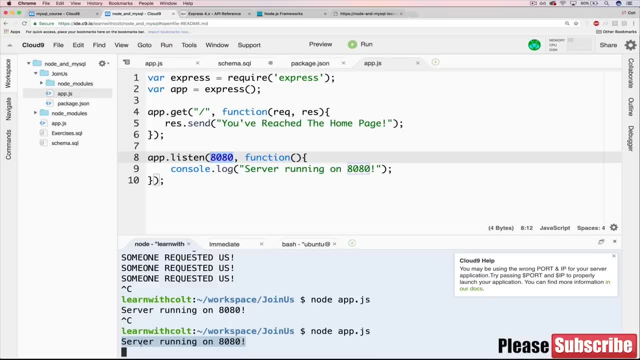 And that corresponds to our server We started down here, So there's an invisible connection here. that's kind of taken care of for us by cloud nine or by any computer, Although your URL would be different if you weren't using cloud nine, of course. 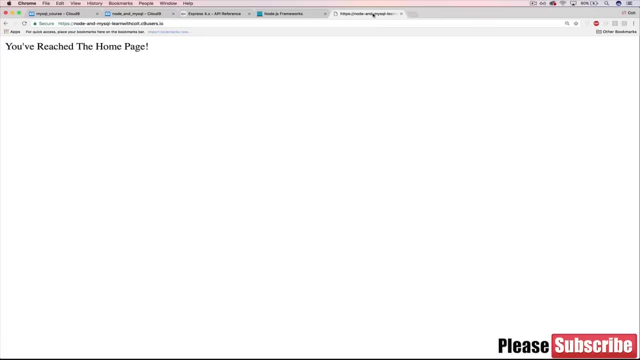 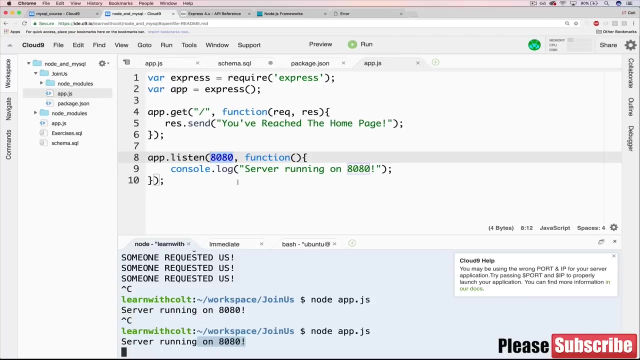 But whatever we're running Here are server. It's waiting and listening for a request coming in. Then we write code that differentiates between something like log out, Let's do log in. We don't have any code expecting login, so that's why we get an error. 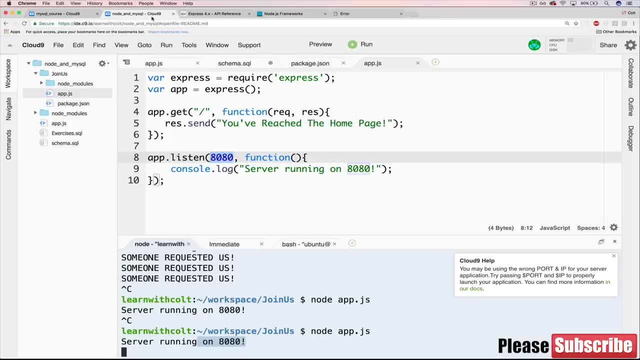 It says: cannot get login. I don't. it's basically our server saying: I don't know what you're talking about. All that our app knows about is slash. That's the only thing it will respond with. Oh, I know that. Let me give you that. 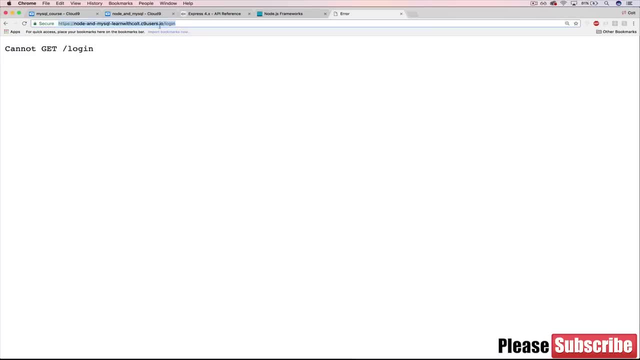 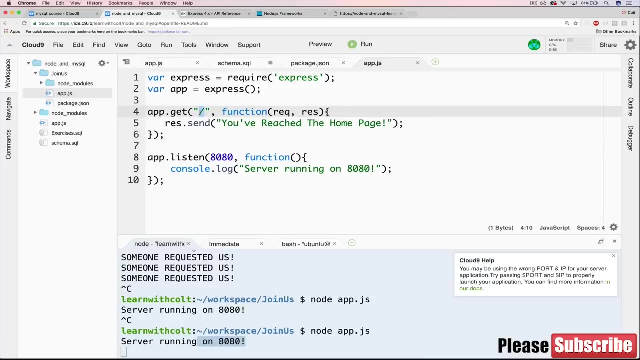 It's you've reached the home page, Otherwise we get, Cannot get, whatever we do. but we do have this one case where it works: The home page. And again, the typical terminology for this is the route, route, the home route. 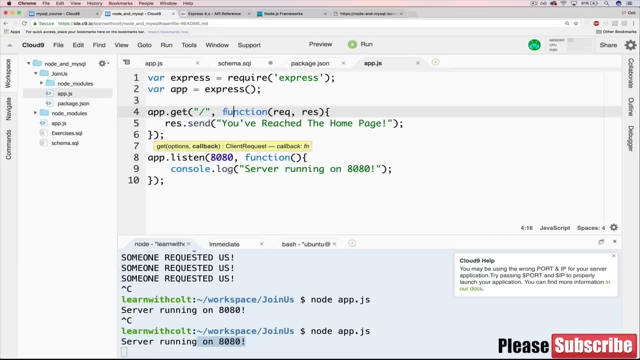 the empty route, basically slash. so app dot get slash, this code runs and all this code does is it responds with. you've reached the home page, One thing that's interesting to take a look at. There's a lot here, but if I do a console dot log request. 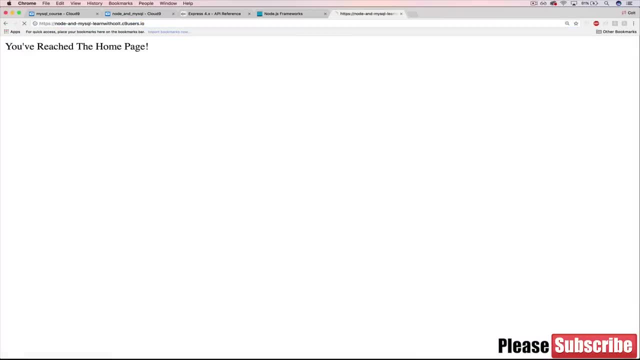 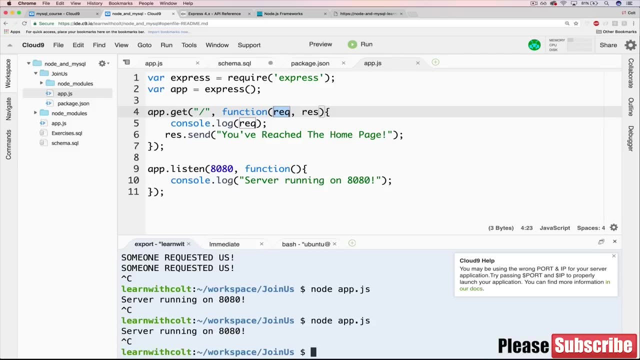 this will contain all the information from the incoming request, from this arrow. There's going to be a lot of stuff in there, So if we take a look, try it again and then make a request, I'll refresh it by clicking over here. We got printed out this giant thing. 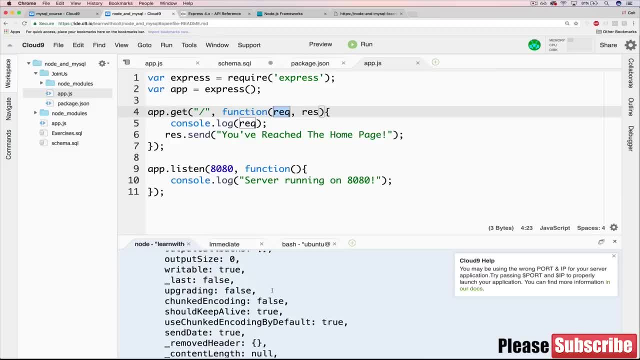 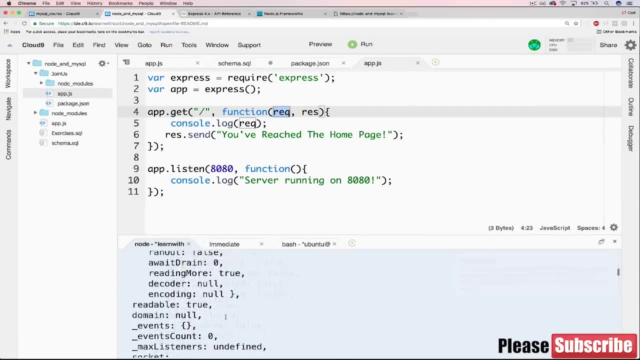 This is all the information contained In that request. So all of this is put together by Express. It's handled for us. Let's see if there's anything interesting to take a look at. Basically, I can't find anything terribly interesting, or that would be. 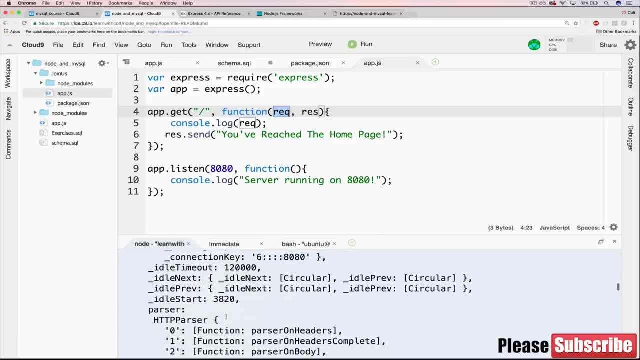 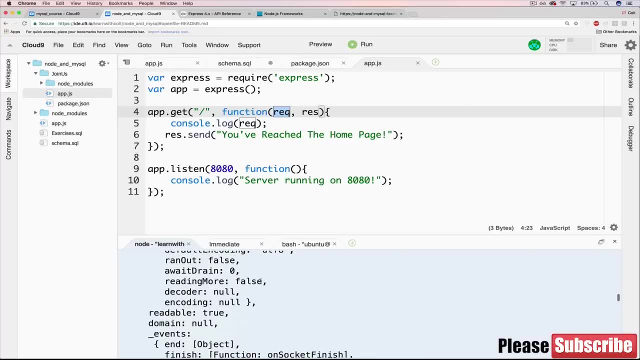 very useful without me having to explain a ton of other stuff, But this contains all the information. Really, you only get one or two things usually that you care about in here. This is all behind the scenes stuff that it works with. With that said, when we make our request, that is sending our email when we type it. 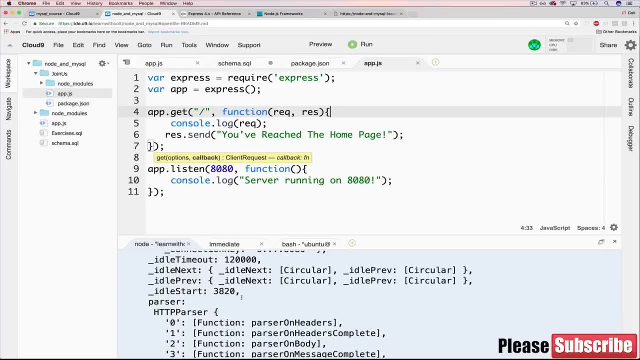 into a form And hit submit. that email will be contained in a request somewhere and we'll need to pull it out, which we'll get there at some point. All right, Next up, we're continuing on with this, but we're going to add a couple other routes. 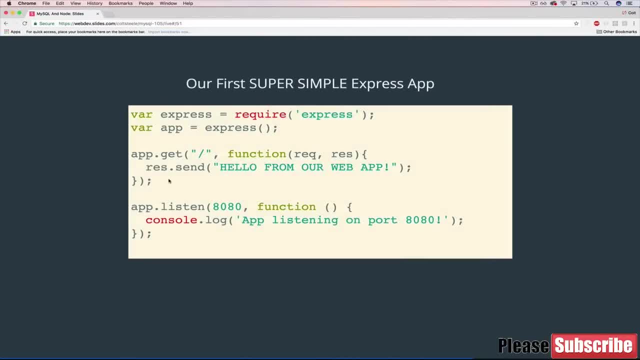 OK, welcome back. So in the last section we saw the syntax to add a single route to an Express app. Our app has one URL that you can request to get a response. Everything else, we get that error message that says cannot get. and then whatever you tried to get, whatever you tried to request, 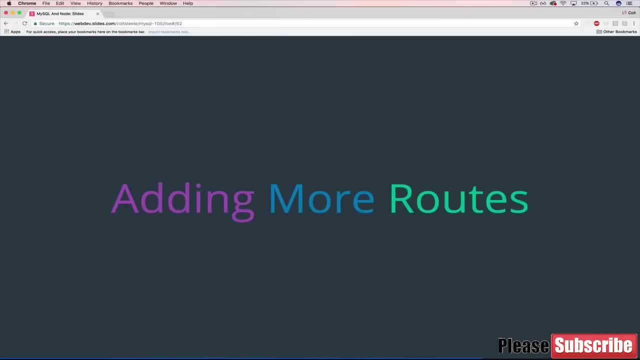 So we'll try fixing that. now We're going to add some more routes, So the first one we'll do is going to be silly. It's a joke route. When you go to slash joke, it just gives you a joke rather than just doing hello. 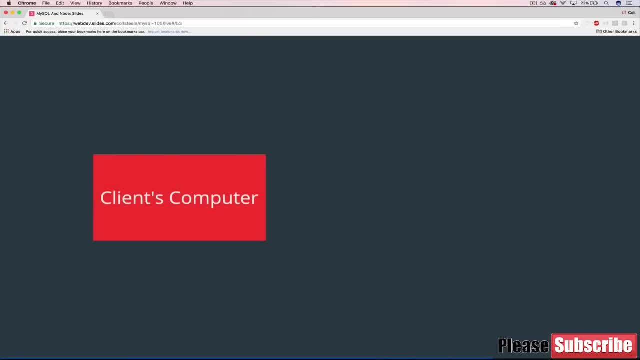 or hi or goodbye, or doing a joke. So when we request from a computer or from a phone event to our URL and then we have our Express app that we're requesting, this time our request is: hey, I would like the slash joke page. 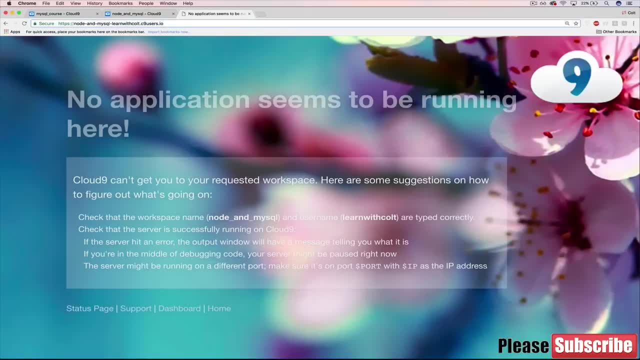 So that's like this: Rather than just hitting enter here, we would go to slash joke. And yeah, you're usually not typing these URLs manually, You're clicking on links, So maybe there would be a link that takes us to slash joke, just as there are links. 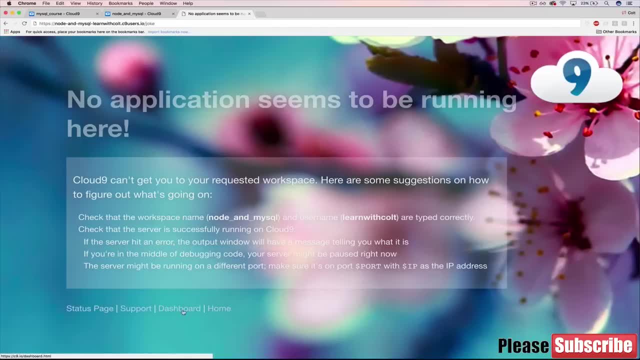 down here. this is an error page for Cloud9, but there are links Each one takes us to. this one is C9.io- slash support. You can see that in the bottom left, very tiny. here you can see slash support. So there's code that is listening. 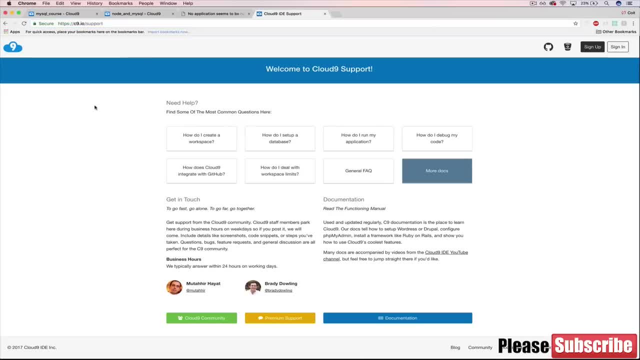 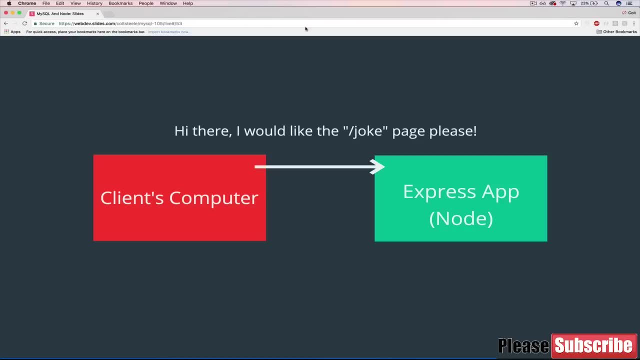 It's taking the slash support and it's figuring out: oh, we need to show the support page that need help, All these buttons on support, Anyways. so we're going to ask for a slash joke. Our Express app is going to say: sure thing. 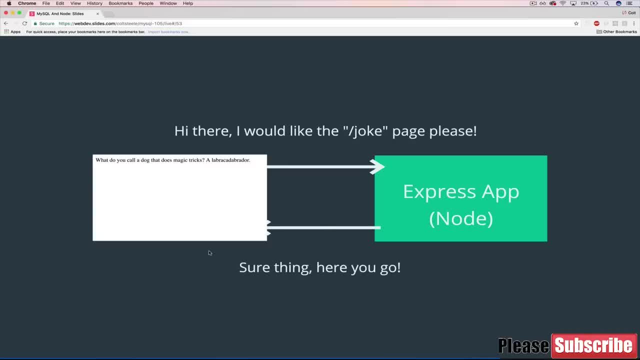 Here you go And send back a really stupid joke. What do you call a dog that does magic tricks? A Labra Cadabra door. I had to pick something that is politically neutral. It's not going to offend anybody, so we're just going with Labra Cadabra door. 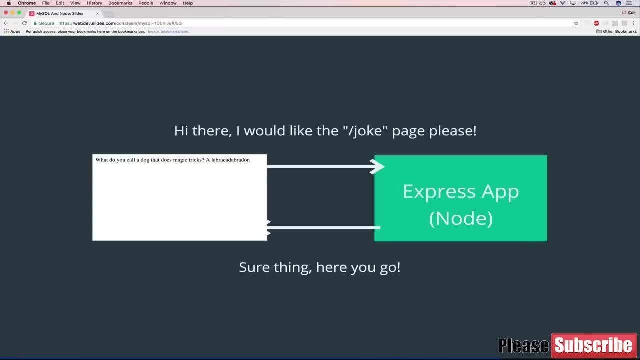 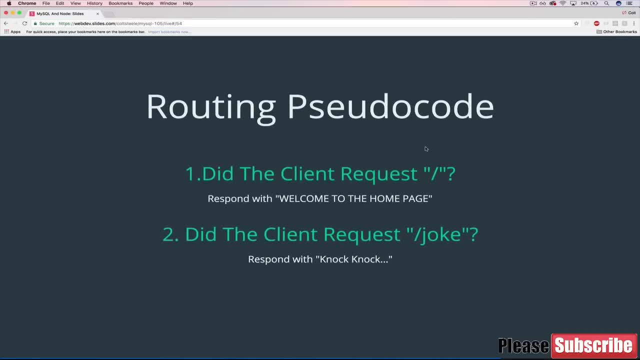 So to implement that, it's very similar to what we've done. We just basically duplicate the code we have, except we change the route, the string of what we're trying to match. So basically, in our appjs file we'll have two questions which are pseudocode. 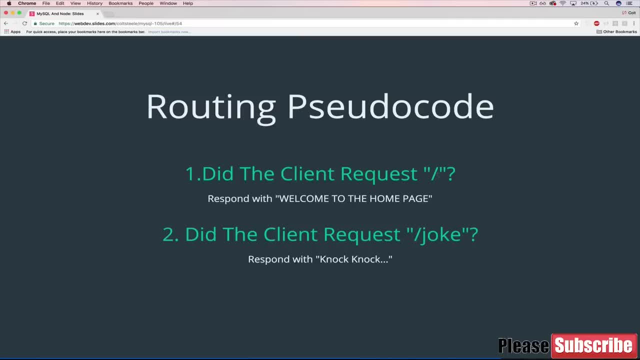 The first one is: did the client request a slash? That's what we already have. If they did respond with welcome to the home page, then we'll also have did the client request Slash joke. And if they did respond with knock knock. 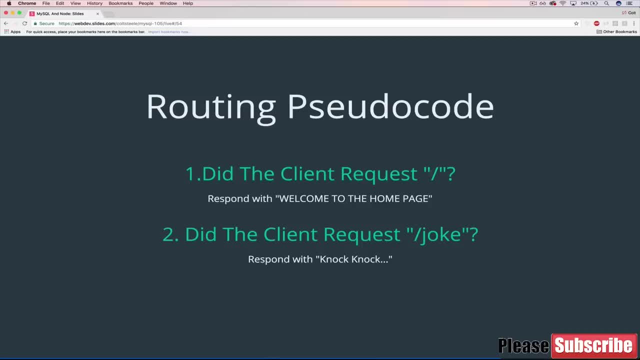 So only one of these is going to run every request, because you can't send a request that is simultaneously to slash and slash joke. So we get one response depending on what we request. So, without further ado, this is all we have to do. 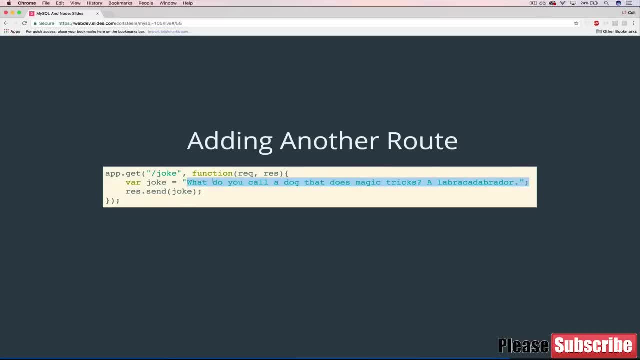 I apologize, It's kind of long because the joke is long, Otherwise the code is pretty short. appget slash joke function request response. And then in here we just have to say: let's have a joke variable equal to our dumb joke. 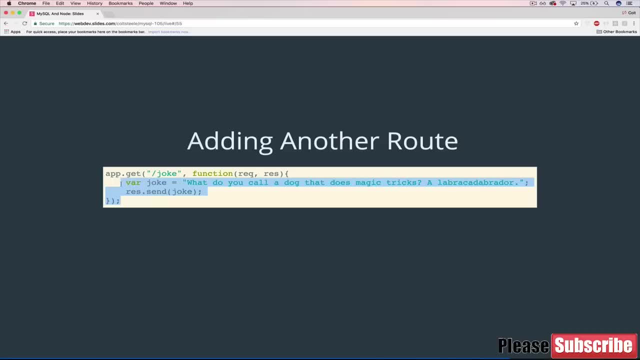 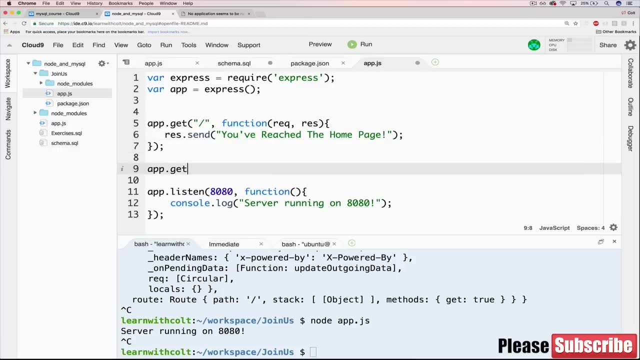 And then we're doing a ressend joke. So if we compare that over here to our existing route, it's very, very similar. So we'll get used to typing appget. Yeah, that was just terrible, but you do it a lot. 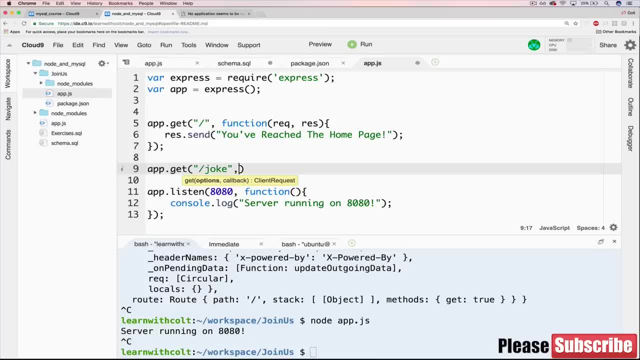 appget And then we'll do joke And that's just something I picked arbitrarily right to have a joke route. When we're actually working with our app, we'll talk about the route we need for join us, But for now we're working with slash joke. request and response. 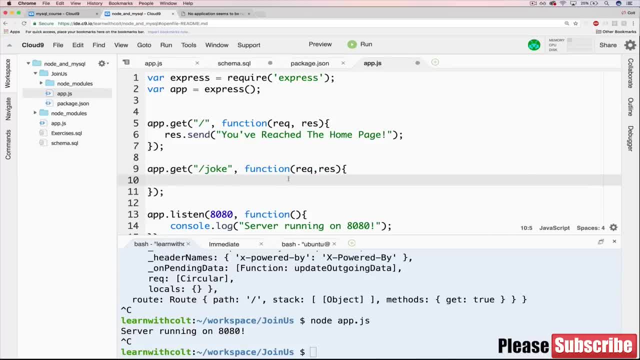 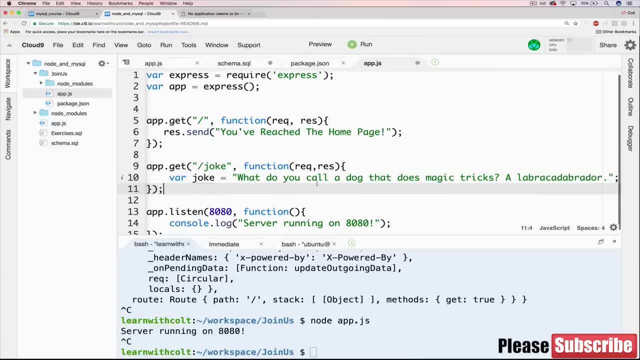 Once again. we can call these whatever we want, but rec and res is pretty standard. Then in here I'm just going to copy the joke. I don't want to make you watch me type that. All right, so we have that and what we can. 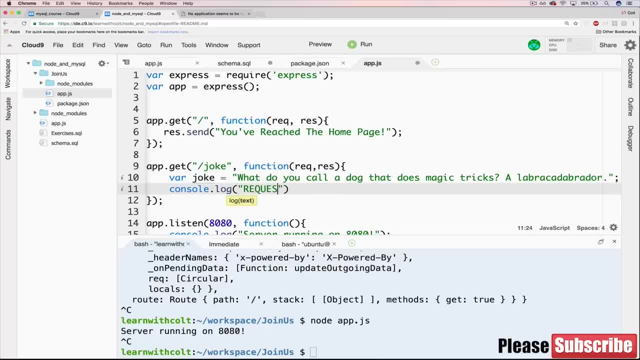 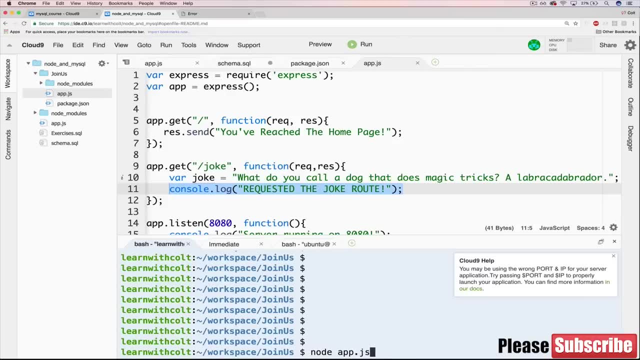 do is the same thing you did earlier. consolelog requested the joke route Quick quiz. What will happen when I run node appjs? When I just run it, nothing will happen, unless we had an error. But what will happen when I make a request to slash joke? 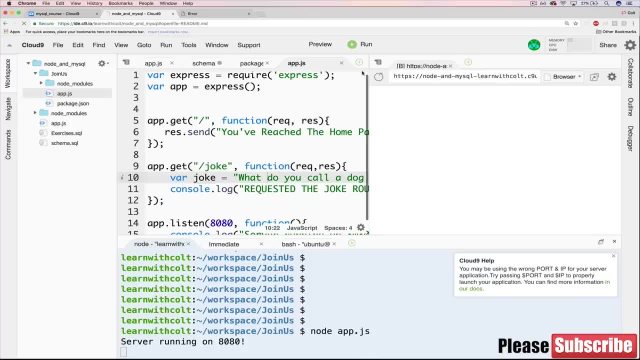 And the easiest way to do that is if I do preview- preview running application- And if I change this to slash joke here- or I could go over here and do it in a separate window. but if I do slash joke and I hit enter, what do you think will happen? 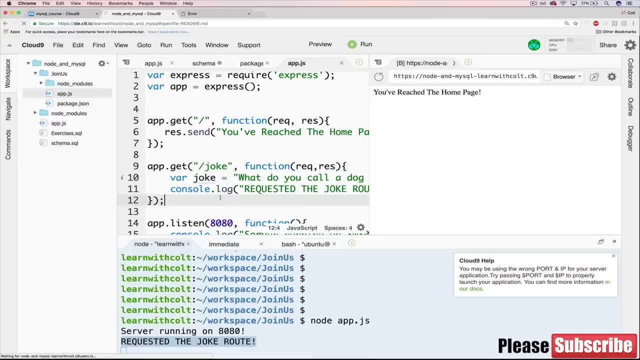 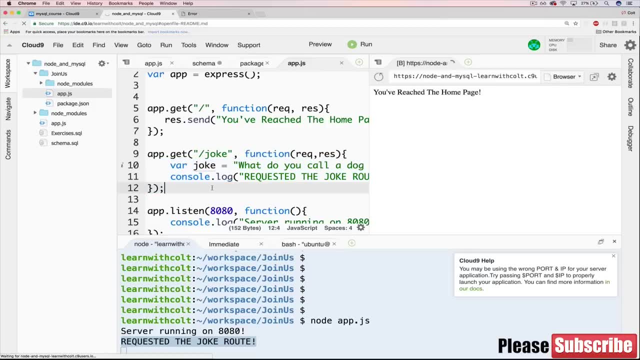 It just keeps spinning and spinning. So we get requested the joke route, which is what we wanted. We consolelogged. That means this route is being hit and we're running this code, But now over here it's still spinning and spinning, spinning and eventually it will. 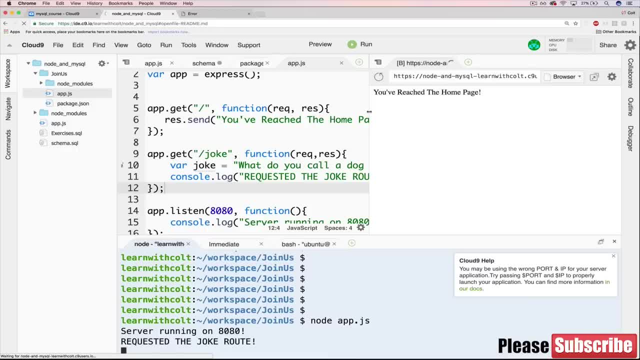 stop and it will give us an error message saying cannot get slash joke. Basically that's saying: you know, I tried, We waited and waited, and waited but there was no response from the server. So the server received it and we did something, but we never sent anything back. 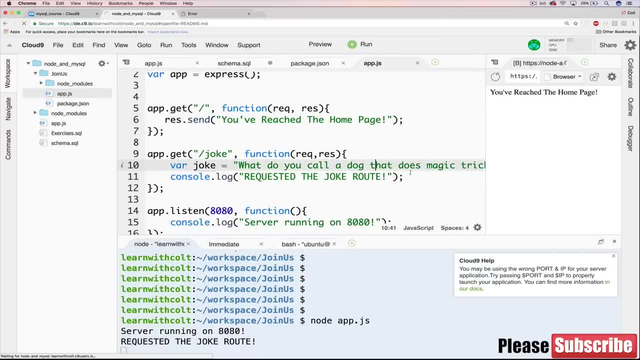 Because we're missing ressend. So very simple remedy. We can have this consolelog if we want it, but it serves its purpose. Now let's do a ressend and all we want to send is the joke. OK, so I'm going to stop this one. 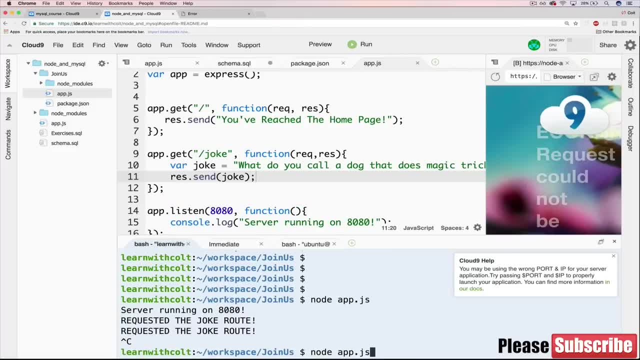 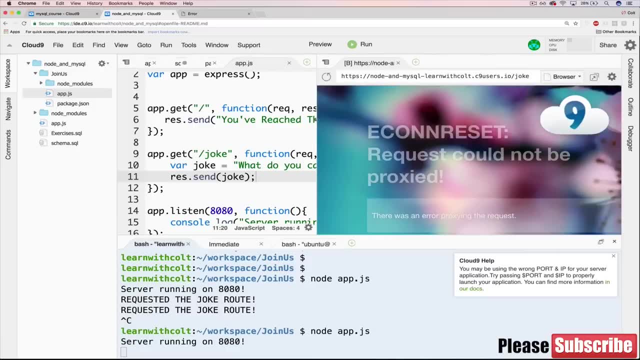 Well, actually I'll just restart the server and that will kill it immediately. Now I'll do node appjs again, make this bigger. I can get it. Go to slash joke and hit enter. And now I get this hilarious joke we've never heard before. 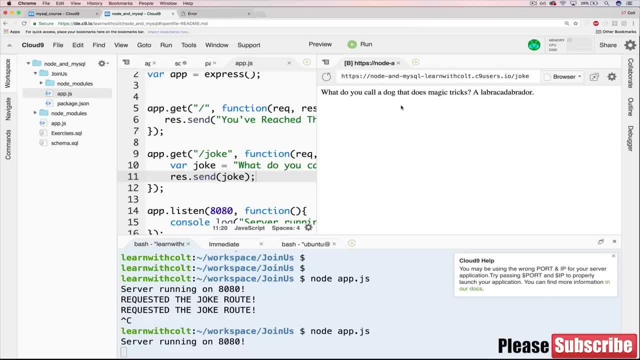 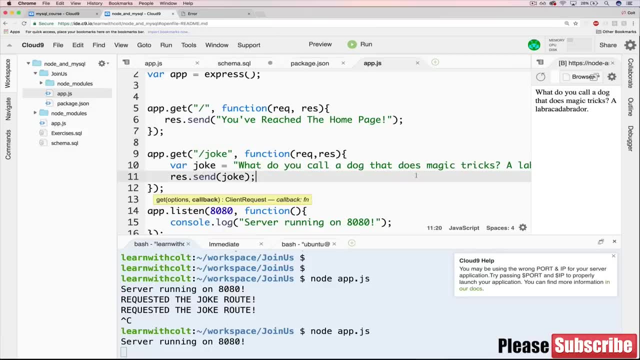 What do you call a dog that does magic tricks? A Labrador? It's pretty good, Pretty good, Whoever came up with that one, And that's it. We have our two routes now, so we could toggle between them. Well, eBay, I don't know where that came from. 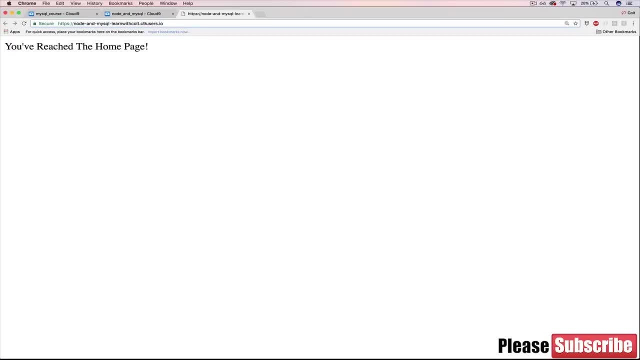 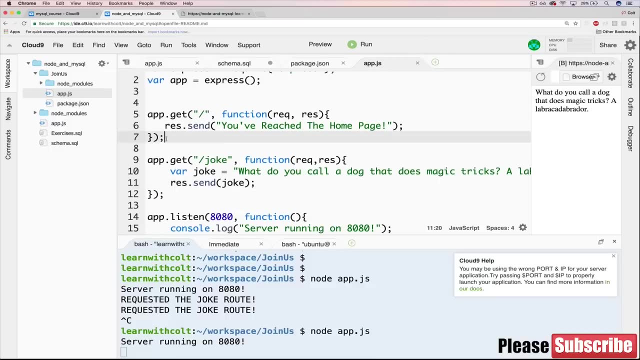 Here we go. So I've got the home route, slash the route route or slash joke, And that's it. So, really, the point here is just to show you you can have two routes, and usually applications have a ton of routes: 10, 20, depending on how complex the application is. 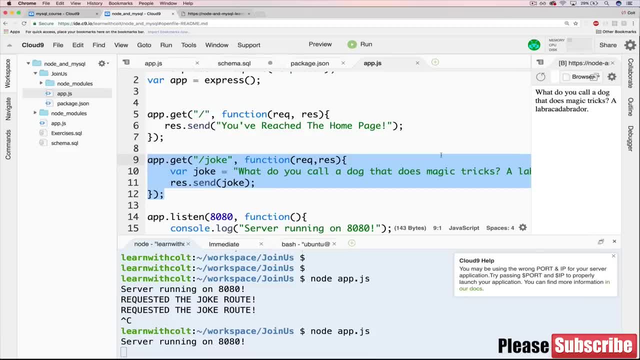 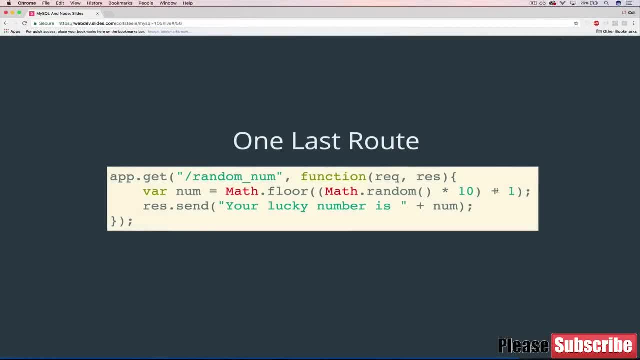 Something like Cloud9 or Udemy might have 50 or 100 different things- Well, hundreds, extreme- But there's a lot of different routes. to wrap up, Let's add one last route. This one is a little different. What it will do is return a random number, randomly generated. 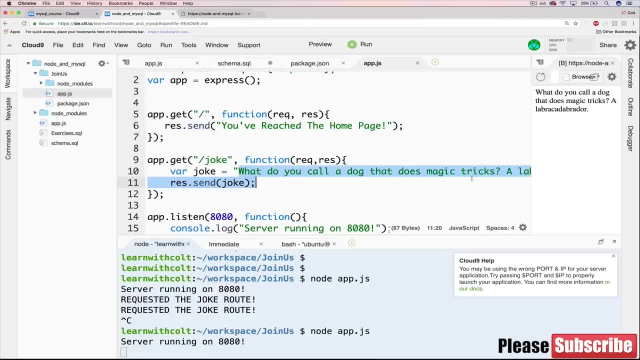 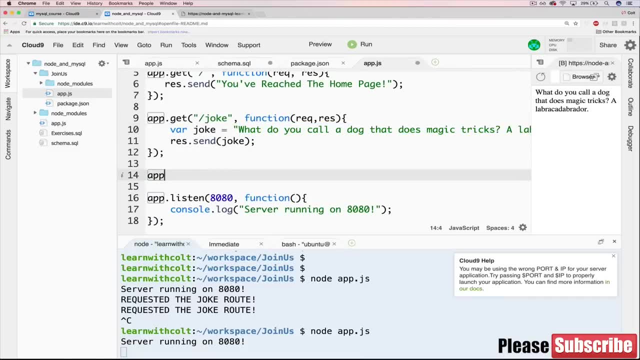 So it's not going to be hardcoded in like you've reached the home page, or what do you call it? A dog that does magic tricks? A Labrador? Haha, very funny joke. Rather than that, it's going to be dynamically generated. 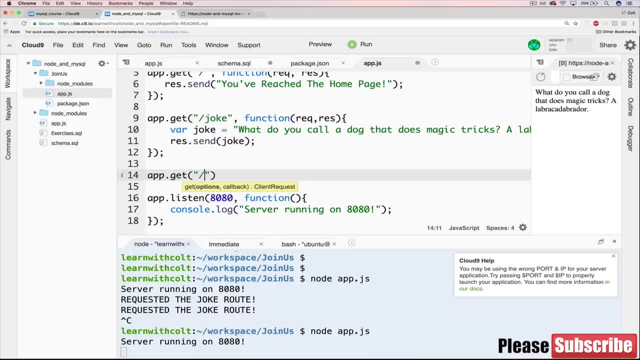 But everything else is the same. So it's appget slash and we're doing random num or number, either one. I did num in the notes comma function, request and response again. So whatever's in here will only be executed whenever someone requests slash random num. 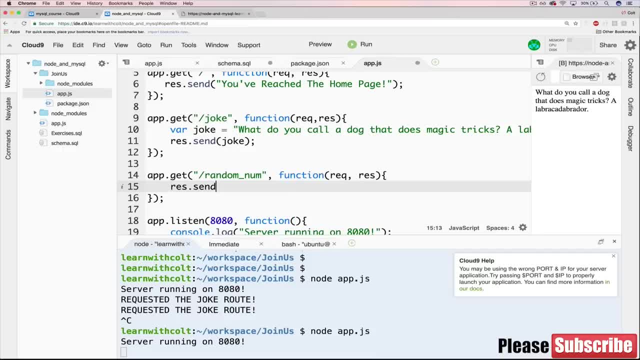 So we'll do our appsend or, excuse me, ressend, And let's just start Just hard coding a number like seven. I'll do it as a string, just to be safe If we restart the server now. Go over here. 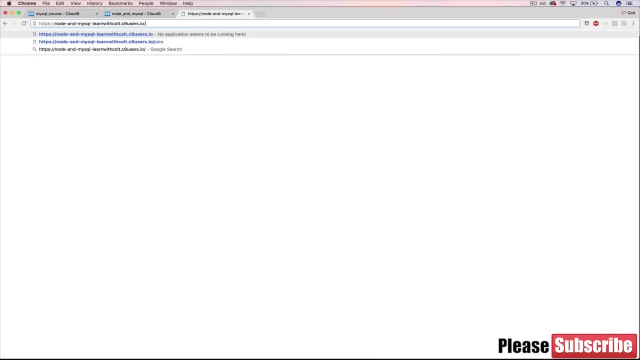 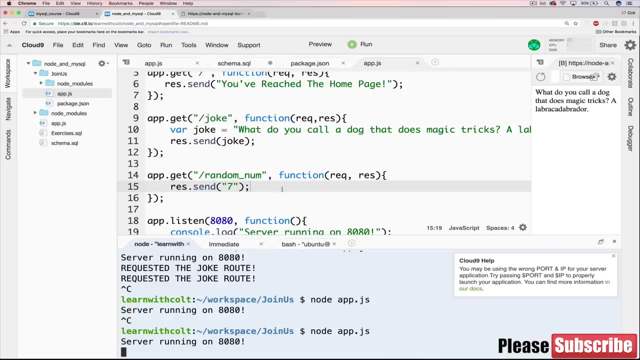 Joke still works, Home still works, But now we have random underscore num and I get the number seven. So now all that's left is to generate a random number, And the way we do it in JavaScript is kind of obnoxious. It's much easier in other languages. 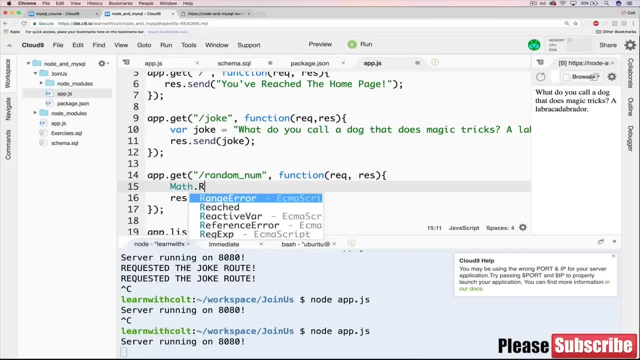 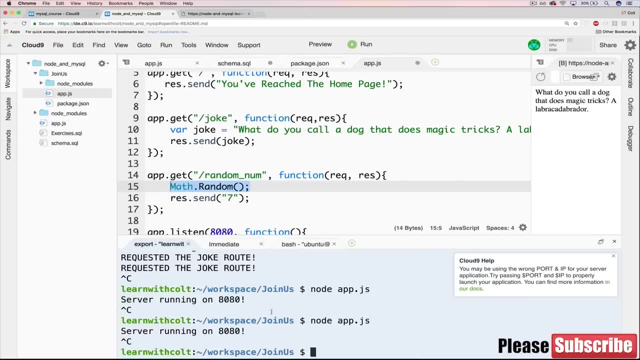 So there is a math Dot random, And what this will do I'll actually just show you right now. If I copy it over, I'm going to stop the server, I'm going to open just regular node, which is not something I've shown you. 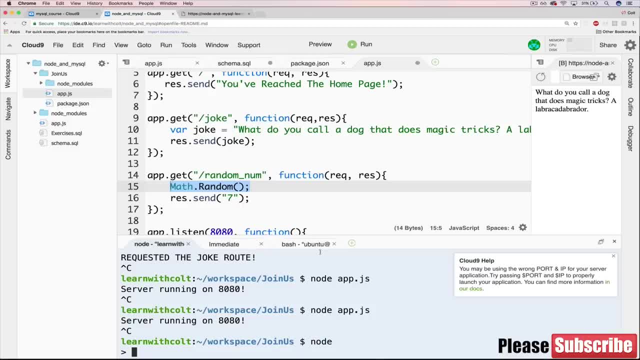 But node has, just like my SQL, has a CLI where you can type things and get a response immediately, Can do one plus one and get to know it has the same thing. If you just type node without a file name, then it opens up a node shell. 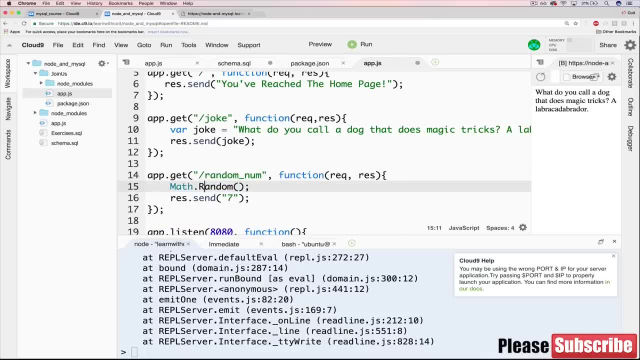 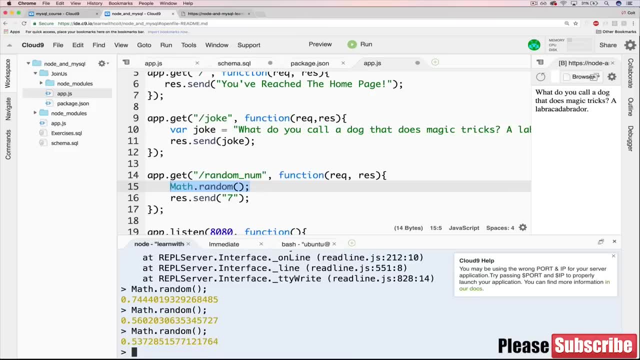 So if I do math dot random and I don't capitalize that are Now I do math dot random, Notice that it gives me a random number between zero and one. It's really annoying that it does it this way, in my opinion. 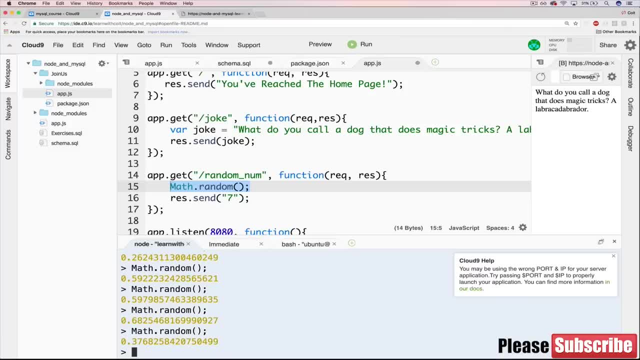 So if we want, let's say something between one and ten. There's a couple of steps involved. We need to generate our math dot random. We need to multiply it by ten. So we'll start with that. OK, so now we're getting one point seven, seven, point four, eight, point six. 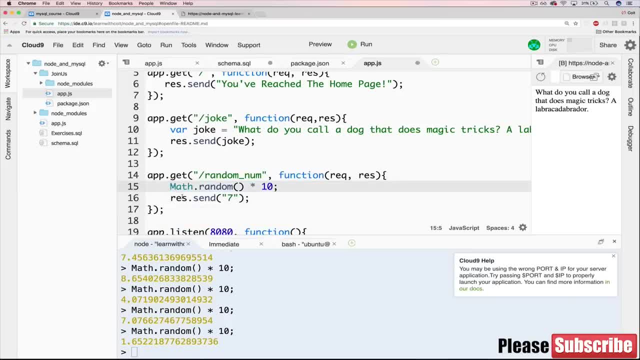 Then what we need to do is get rid of that decimal, So you can either round What's more standard is to do a math dot floor. So what that will do is just chop off the decimals. So we end up with eight, nine, eight, two. 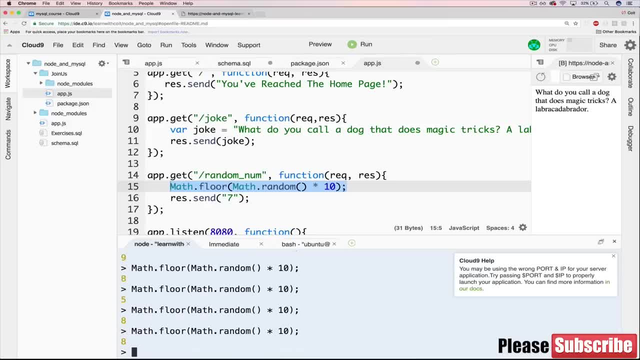 But then we have a problem, which is we never actually hit ten. We're doing a number between zero and nine, which you'll have to trust me, That's how it works. But you can see we have zero here And it's because when we did our original math dot random. this is: 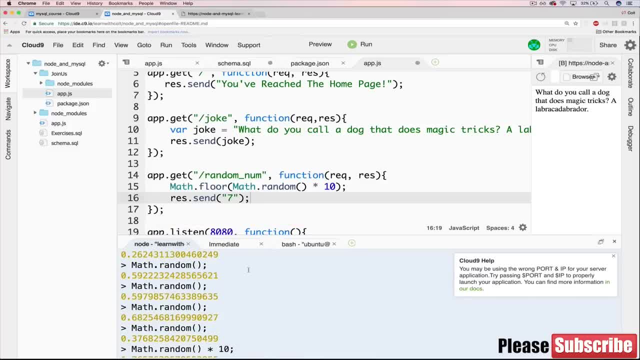 a number between zero and one, non including or not including one. So up to point, nine, nine, nine, nine, nine. So all we want to do is then shift it by one. So it's kind of a lot of work to generate a random number between one and ten. 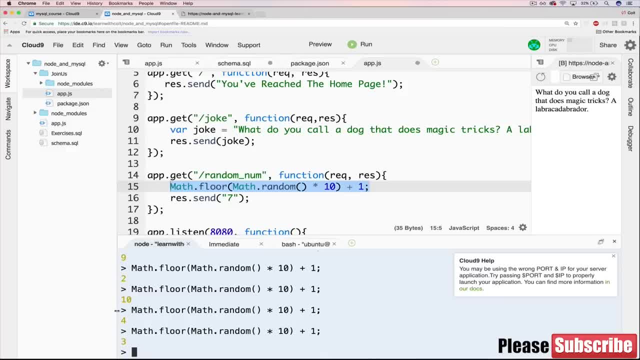 But now we've got it, just to prove. OK, there's a ten, We're in the clear. So now we'll just make that a variable. We'll just call it X, maybe equals. Well, maybe now is a better name. 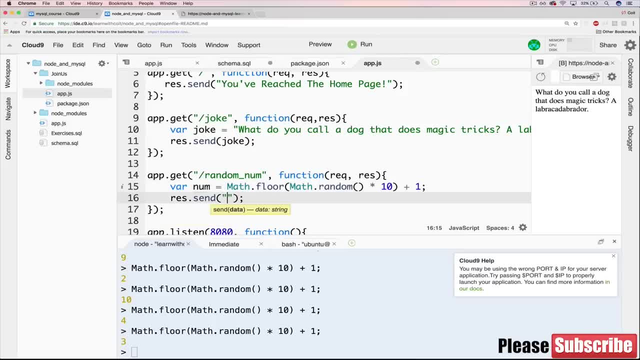 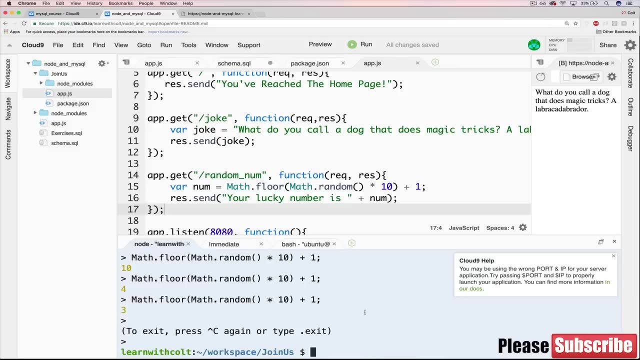 Make it a little clearer, and then we'll just send it back. We'll say You're, and I think I said lucky number is plus No, and that will just concatenate it in there. Let's try it. So to get out of node, we just do control C twice. 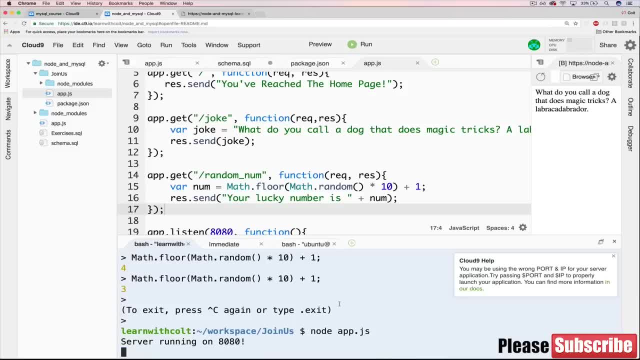 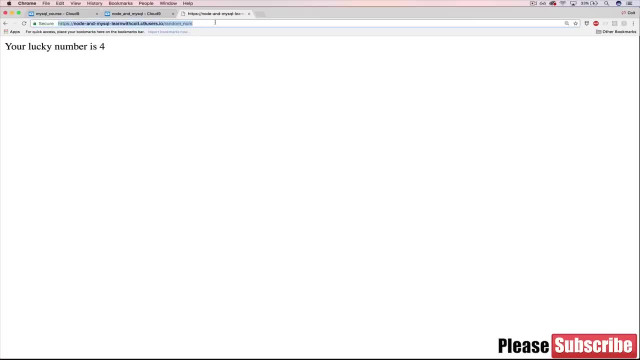 Now we actually execute our app, app dot JS. Now, if I go to random, num says my lucky number is three, now it's ten, now it's eight, eight again for you get the picture. And of course, we still have our home route. 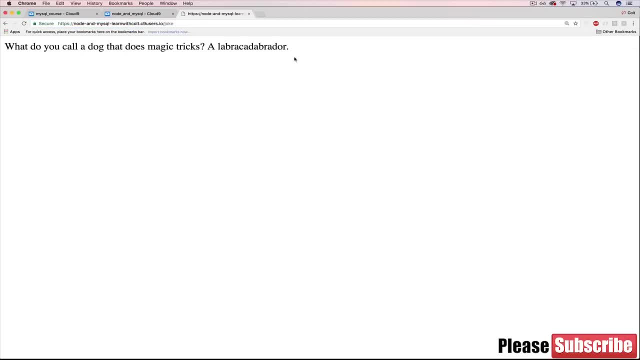 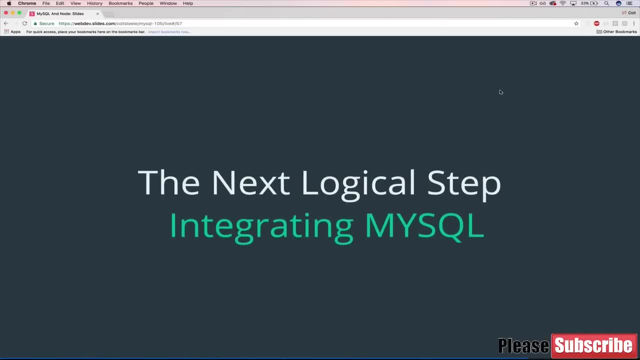 and our refreshingly adorable and hilarious Labrador joke. OK, we're done here, Moving on in our next video to actually integrating my SQL with this Web app. Big step: OK, welcome to this big step. What we're doing next is integrating my SQL into a Web app. 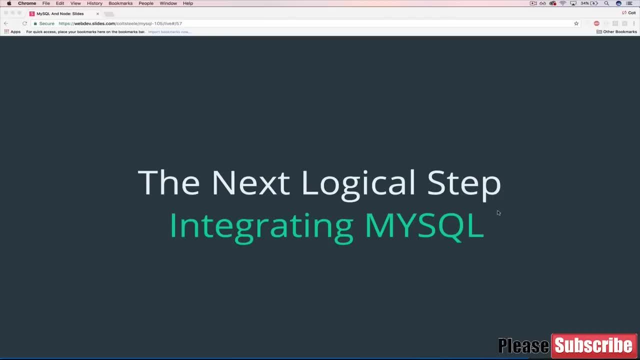 So we saw again how to integrate my SQL with node in a single file. that has nothing to do with the Internet or Web applications or servers or routes where we just inserted five hundred users At once. Now what we're going to do is take our Web app that we've created. 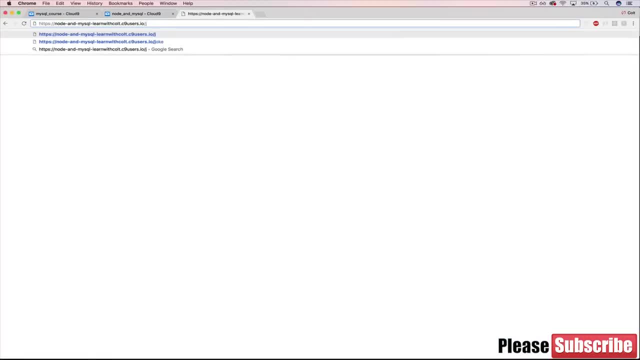 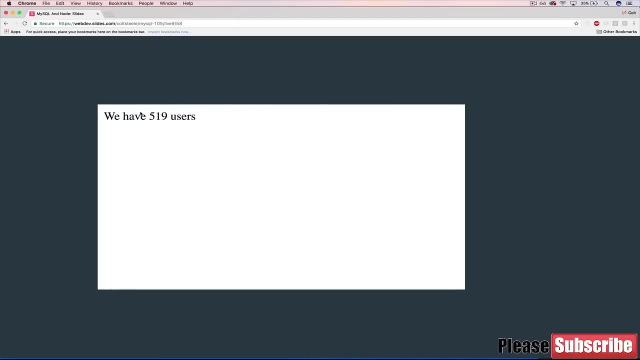 Super simple, unstyled, but something like this: When we go to the home page here right now, it says you've reached the home page. What we're going to try to do is take it to this. We have five hundred nineteen users, and that five hundred nineteen is not hard. 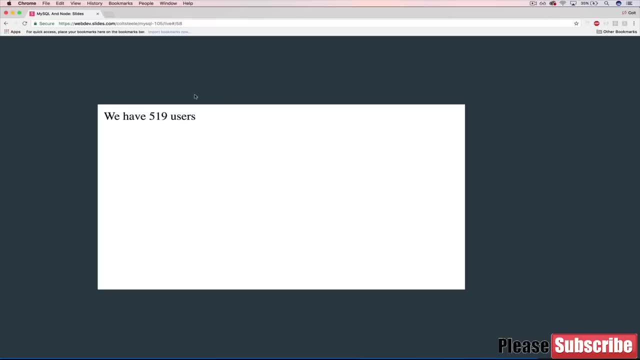 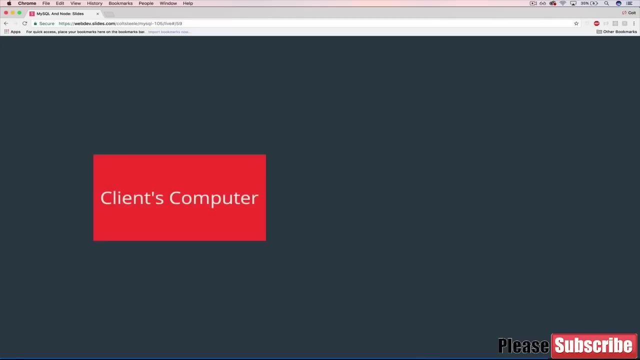 coded in. that's coming from our MySQL database with the five hundred, something that we inserted. So this will change depending on how many users are in our database And we'll see that that works. So to do that we're basically- I have another diagram that took ages to put together- 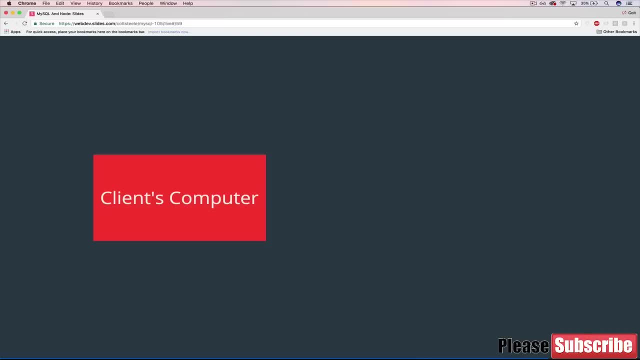 I apologize if it's the colors aren't perfect or there's not nice typography. I wish I was better at that stuff. But here's our trusty red rectangle that represents a client computer. Here's our Express app, This mint green. This time we're requesting the home page. slash the route, route. 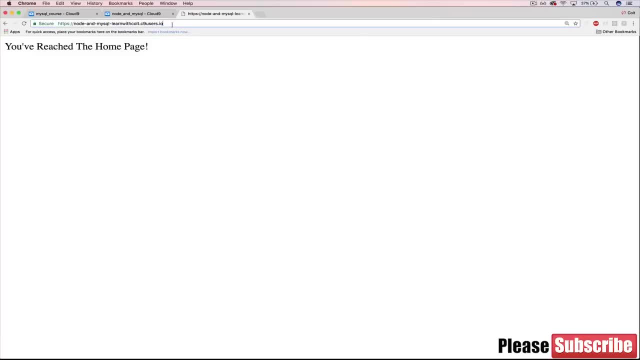 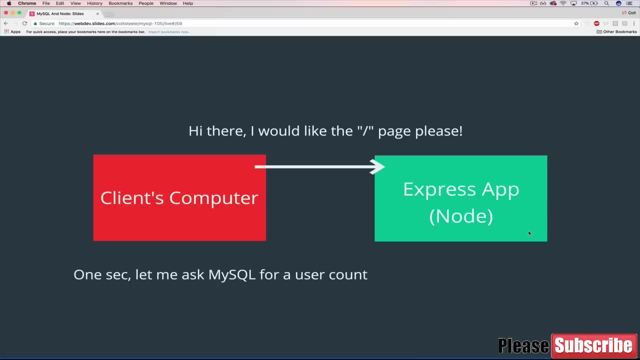 We ask the server for it by going to this URL, hitting enter. The server says: oh, hang on. It says here that I need to ask MySQL for a user account. OK, so MySQL is now involved. This arrow represents the connection between Express and MySQL. 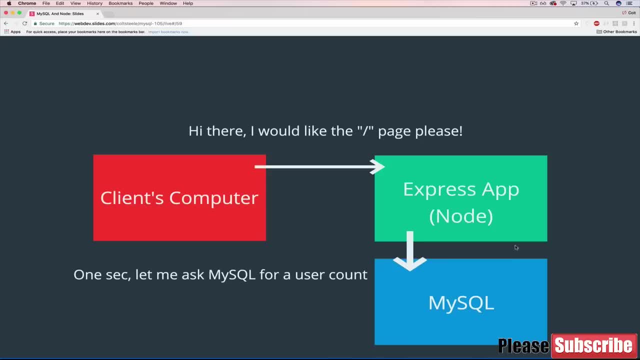 We've already seen how to do that, how to connect MySQL to a JavaScript file. We ask, basically, with a select statement, select count from users. We get a response from MySQL. Hopefully there's not an error. We get a response 519.. 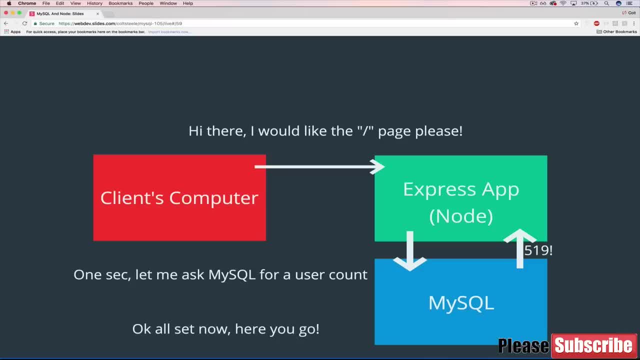 Then our Express app can take that and say: OK, we're all set. Now here is your final result. Here's the page we get. We have 519 users, All right. So there's a couple of steps involved that we need to do. 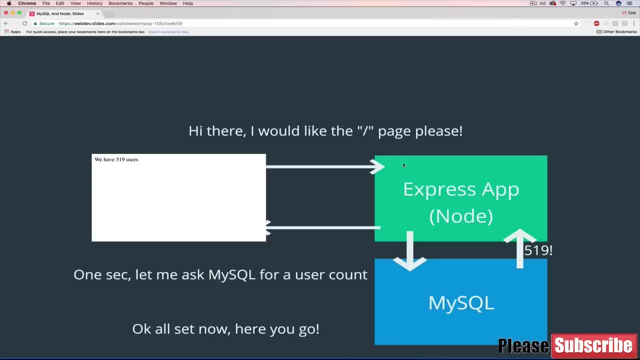 Basically it boils down to: we've already seen how to make a simple route, And in the last section we saw how to connect MySQL to a file. Now we just need to combine them together. So the first thing that we'll do is go over to cloud nine. 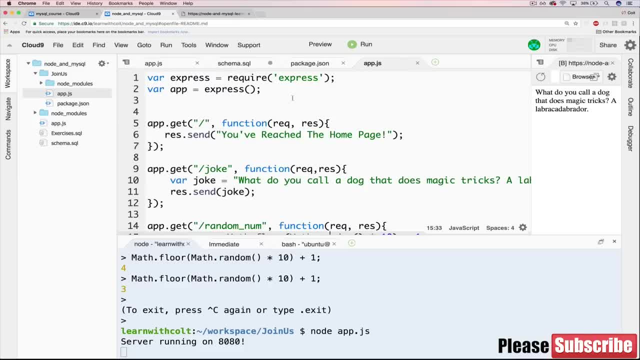 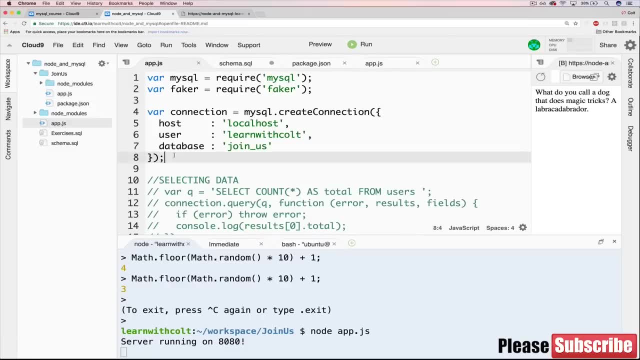 And we need to connect our app, this file, to our MySQL database, And what we can do is just go to our previous app, JS, and just copy this code: for our connection equals MySQL dot- create connection. so I won't make you watch me type this whole thing again. 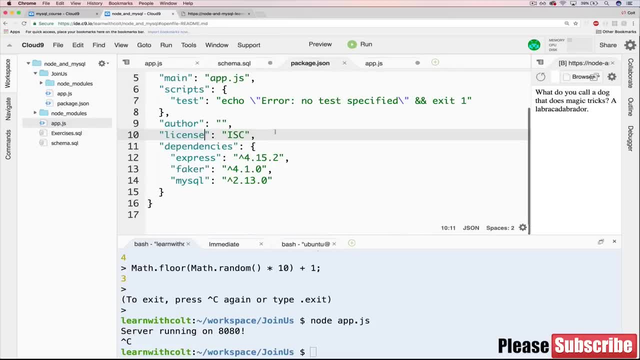 But remember, this is using the MySQL package and we already installed that. earlier You ran NPM: install dash dash, save MySQL. If you didn't do that yet, go ahead and do it so that you see it Here and that inside of our join us. 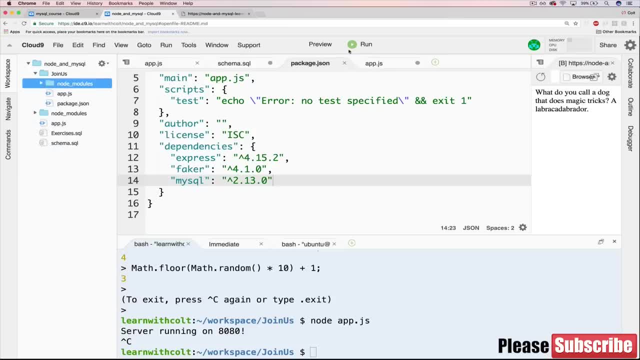 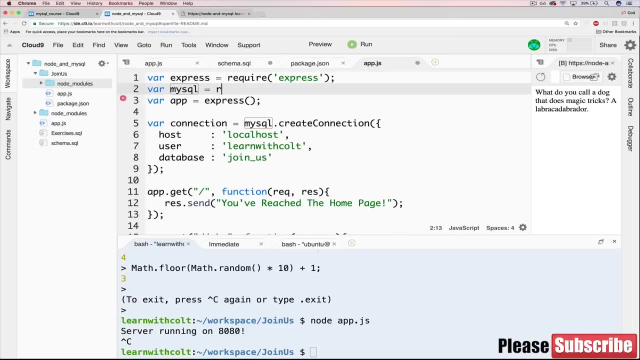 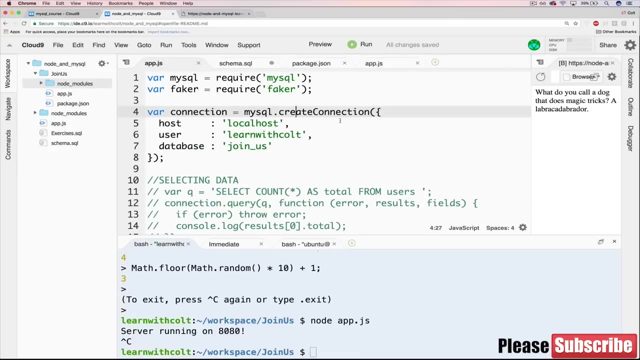 folder. instead of node modules, we have MySQL. We need that, But we're still missing something, which is we need to require it for MySQL. equals require MySQL. so this is all review. We did it earlier when we made our seed data that inserted 500 users. 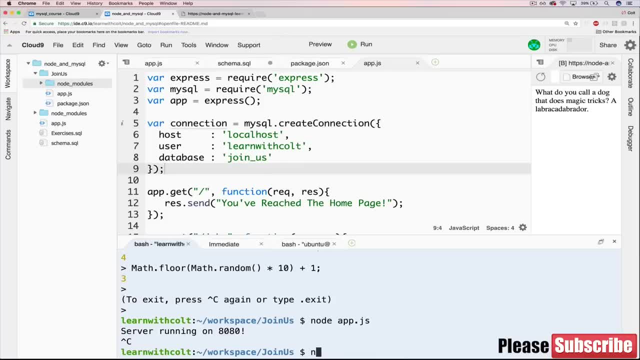 So we've got this and let's just make sure that that works without problem. So we'll just start node app dot JS. Everything looks OK, All right, So now we can focus on interacting with the database, now that we've connected to it. 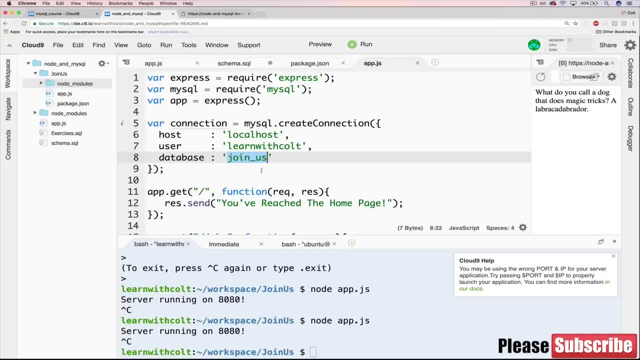 But just to reiterate, this database name needs to be the name of the database inside of your MySQL server that you created with the users table. So it's the same as what we were doing earlier If you've been following along. if you named it something else, this has to match. 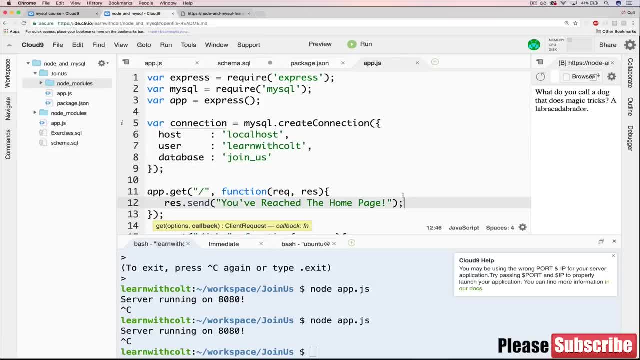 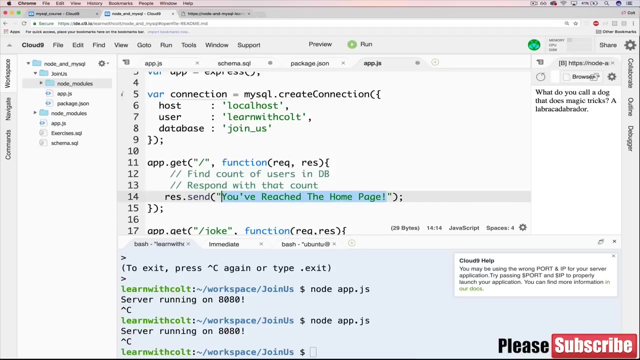 So what we're going to do is, instead of you've reached the home page, we want to find Count of users in database And then we want to respond with that count. So we've got a res dot send. Eventually, what we're hoping to do is have something like we have plus count. 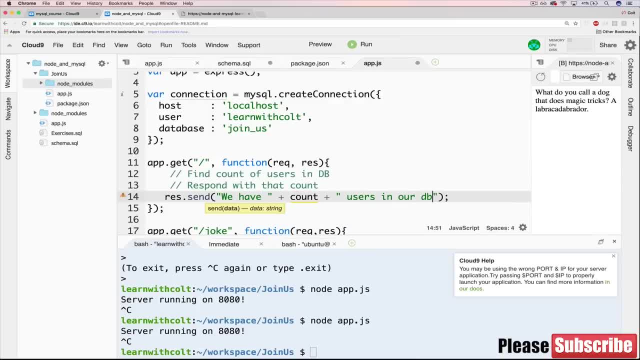 Plus users in our database, or something stupid like that. that's what we're hoping to do. Of course, right now we don't have this count variable, So that's what we need to aim to get to, So I'll start by commenting that rest send out. 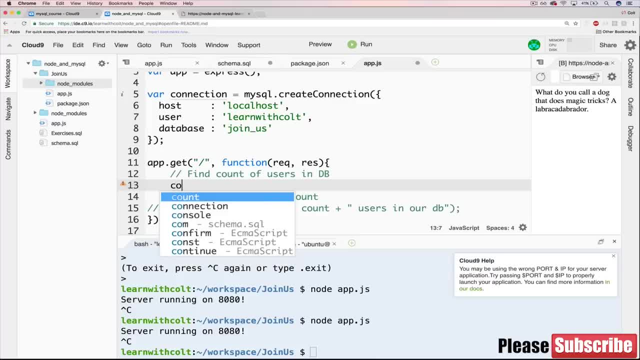 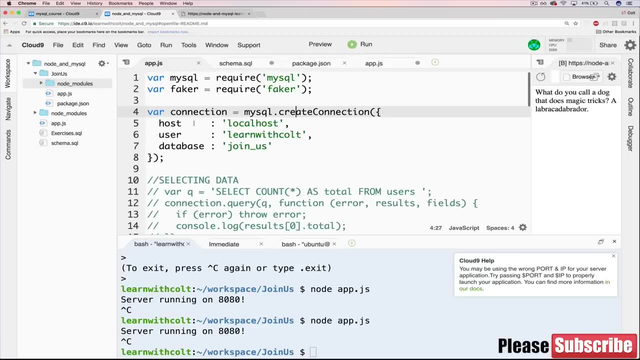 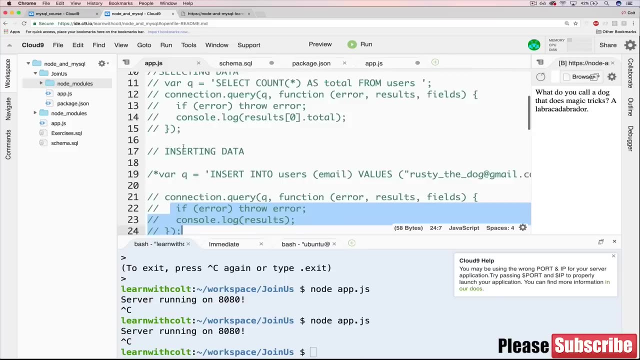 So to find the count of our users in our database, we need to do a connection dot query, which we've done before, Remember, it's all the stuff we were doing over here. Connection query, Connection query, connection query. And what is the query you want to write? 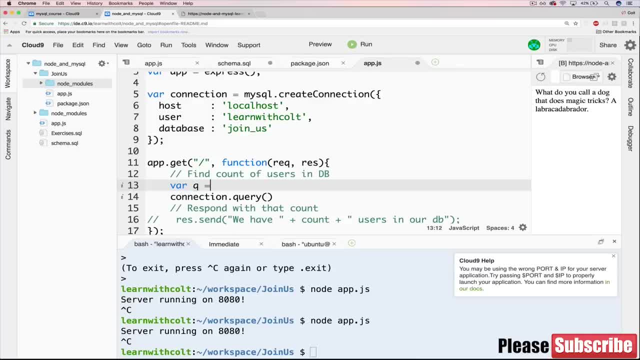 Let's do it in a separate variable. So far I'll just do Q again equals a string, Select, count star from users, just like that. If we were to just copy it, go over to our MySQL, we get 500.. Okay, so that's what we're hoping to get. 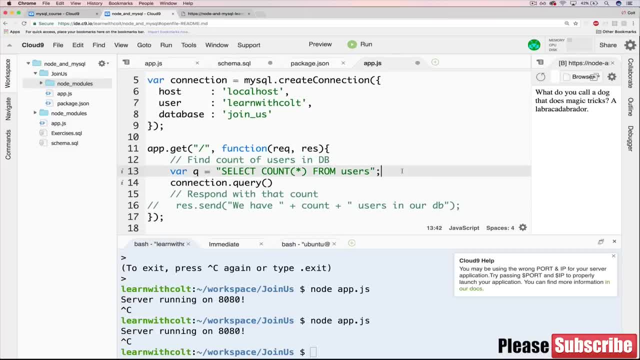 But of course through JavaScript. So we've got our query written as a string. Now we just pass it in connection query, Then we add in that fun callback or we have error and let's call it results, OK. so whatever code is in here will only run when two things happen. 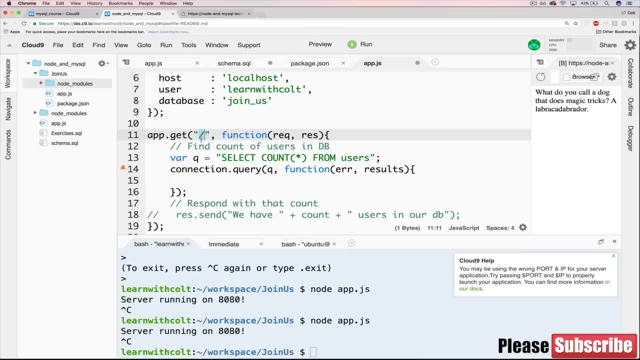 First, when somebody requests slash, then we have to wait for this connection to run the query, which is select count from users. So then, when that is done, whether it worked or not, this code runs and it will either be an error. 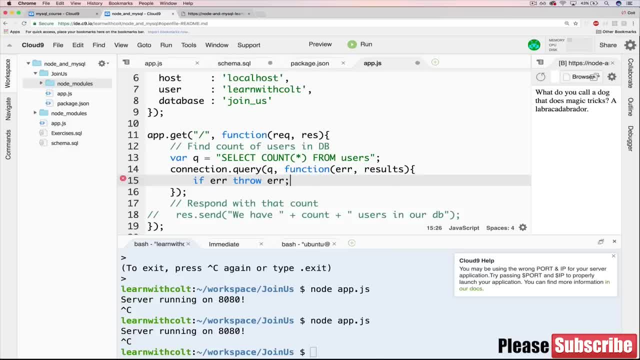 So we can add our if error throw error, which is not actually a great thing to do in a web application. What would probably be better is to say: if there's an error, what do we want to do, Redirect the user to a different page, or 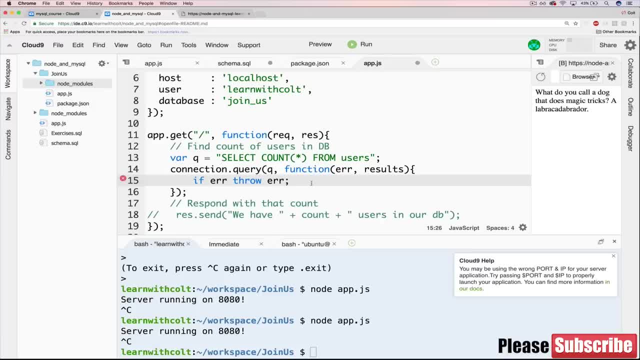 send them a different response, which we can see how to do in a little bit, But we're just going to leave it as that, to keep it short, And then otherwise let's do a consolelog results And just see- oh, just see- what we get. 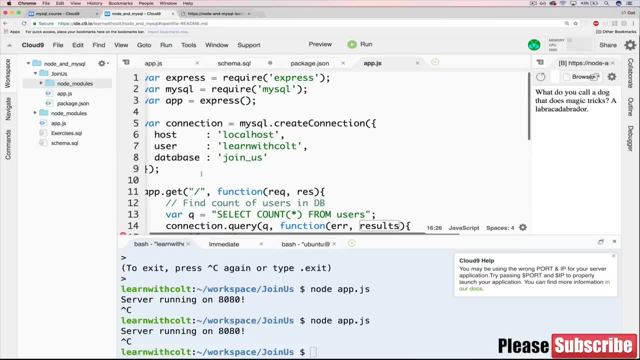 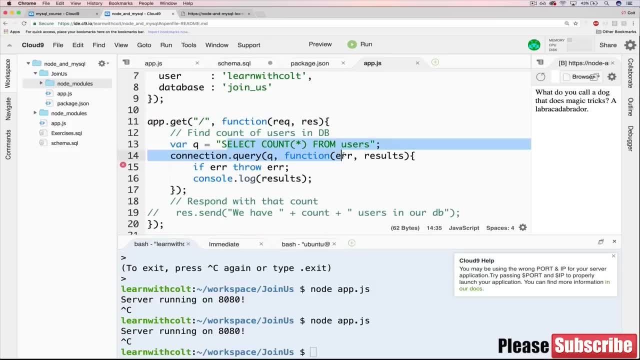 OK, so again to go over this connected to our database. then only when somebody requests slash are we trying to select count from users. We could do it inside of joke if we wanted to, or random num, But the way that our app is going to work. 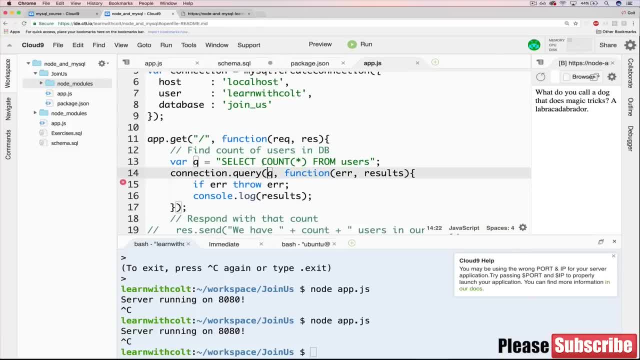 the home route. when we go to the home page we see you know welcome or join us, Join the 519 users or whatever it is, And then there's a form at the bottom. So we're just going to do it on the home route. 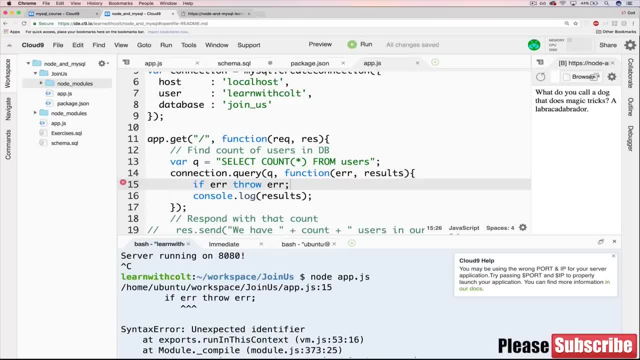 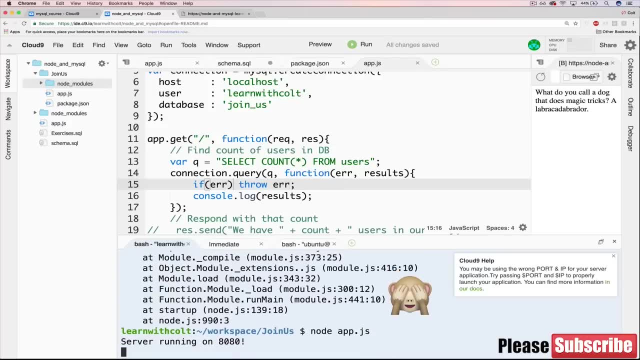 Let's see what happens. if I try running node app JS, Looks like we have a syntax error And that is because we're missing parentheses around. error there. OK, now we're good to go. Now, if I try and just go to the home route, not joke, well, joke will work just. 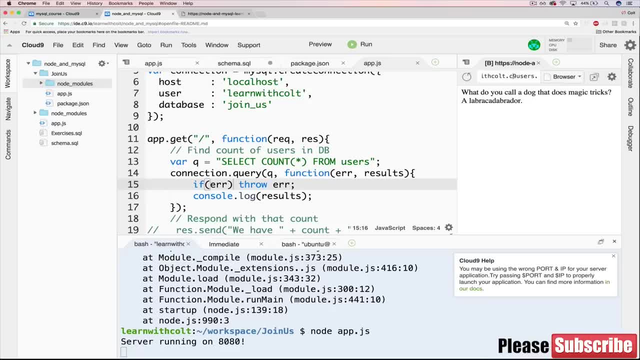 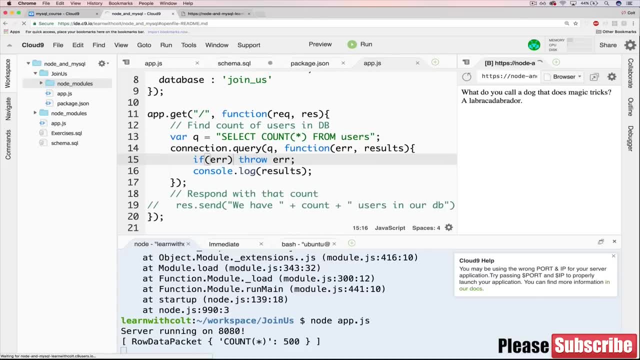 fine, but if I try and go to the home route, what do you think will happen? And the answer is that we're not responding with anything, assuming we don't get an error. We're not actually responding with any rest send, So we're not going to see anything over here. 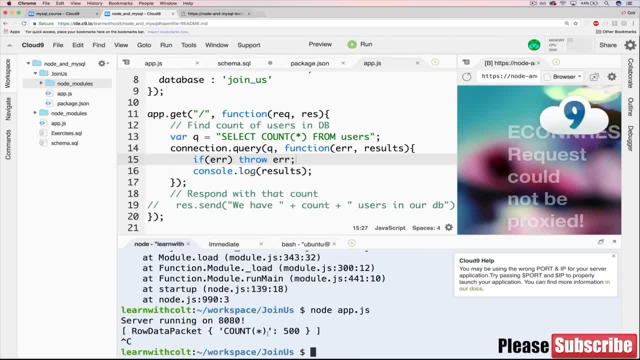 It just waits and waits, and waits until it gives up. So I'll stop it here. But notice, we get this row data packet, a single array with one item in it, So we're going to want to do result zero. And then what is nicer is if we give it that as 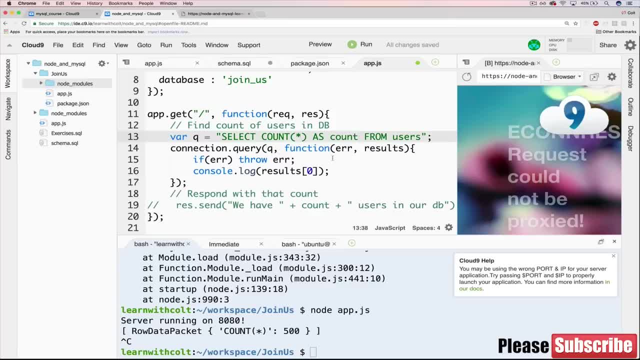 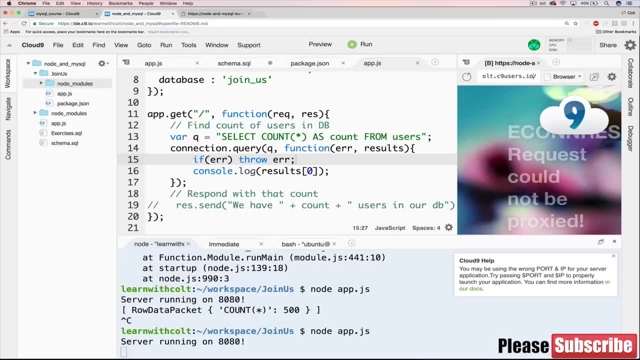 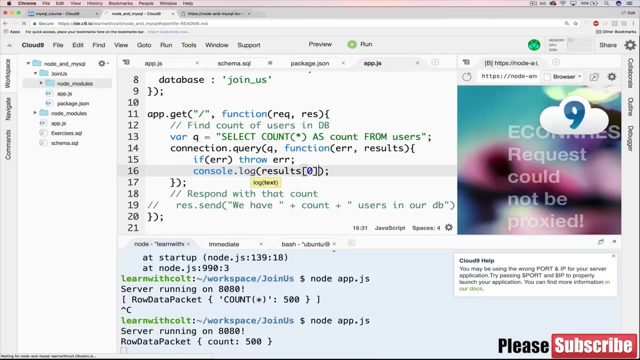 alias. so we'll say select count as count, just like that. So now if I start the server up again and I refresh the page, this time we get row data. packet count is equal to 500 inside of an object. So all I need to do is do dot count. 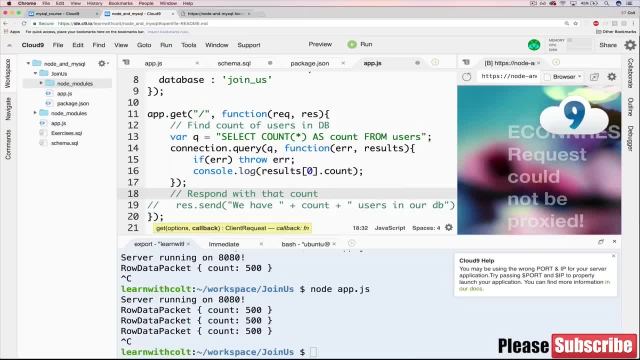 So this will print 500 now. So let's save it to a variable, var. We'll just call it count as well. So now we have a variable with the count in it. So then the last step: I'm going to get rid. 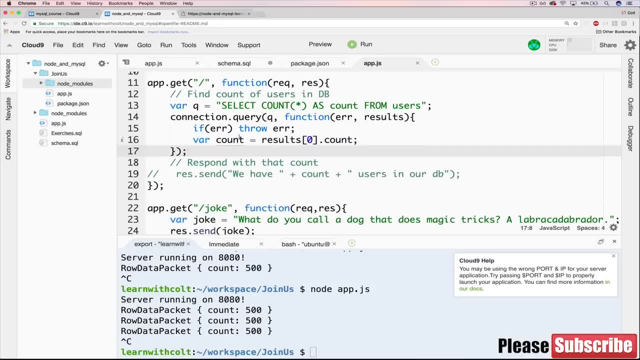 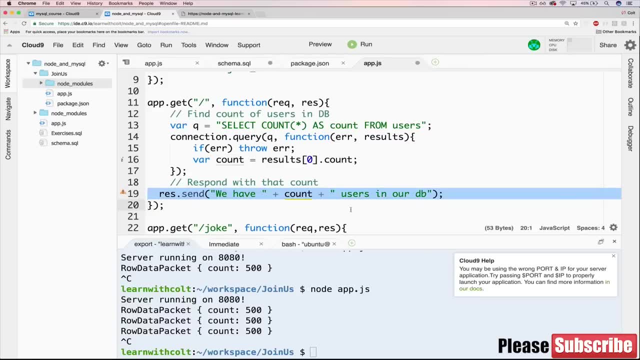 of the in here and just work over here. But now that we have our data coming back from the query, we're going to want to do a res dot send. Now, something that tricks people up, trips people up, is when you're working. 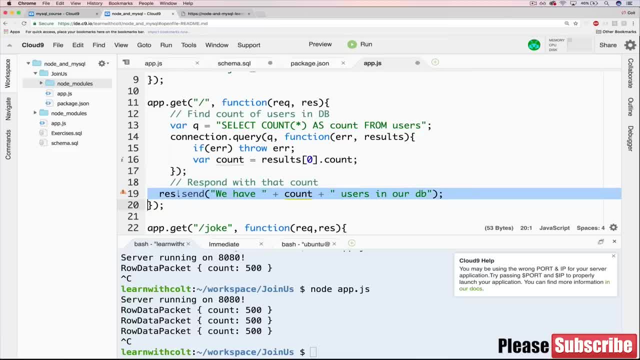 with callbacks like this, it might seem like this code is going to run after this, but in fact, we have no guarantee of that. What we want to do instead is only run it inside of this callback. So this is a very common pattern in JavaScript and in Node. 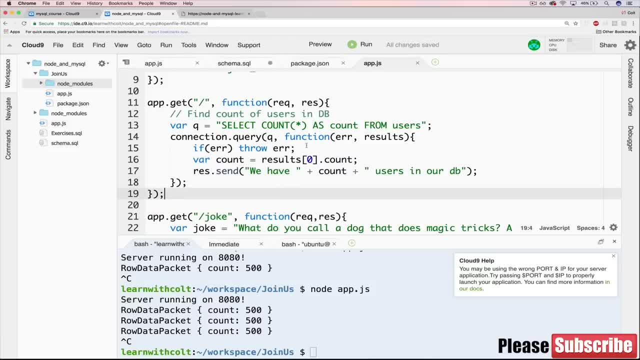 in particular is that you have these nested callbacks and it can get out of control sometimes, or something called callback hell, But this isn't too bad. It's not bad at all. So we have our route app, dot get. When this route is hit, run all of this code inside of there. 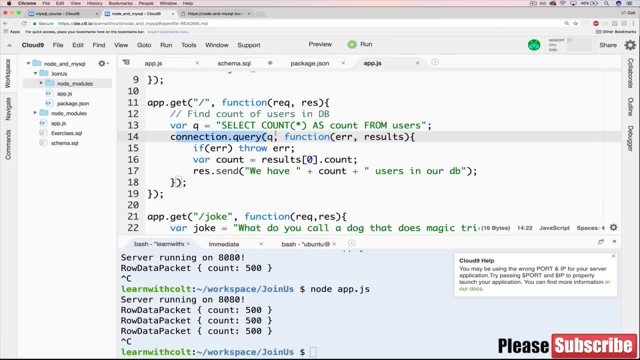 We're defining a query and we're doing that query, and it takes time. It might take half a second, although that would be pretty long, but it might take a tenth of a second or something- And so what we want to do is wait until it comes back and run this code. 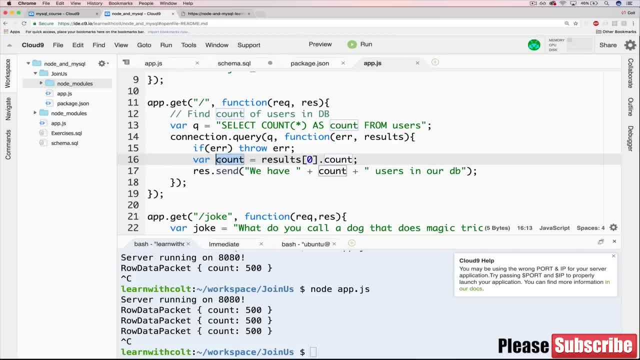 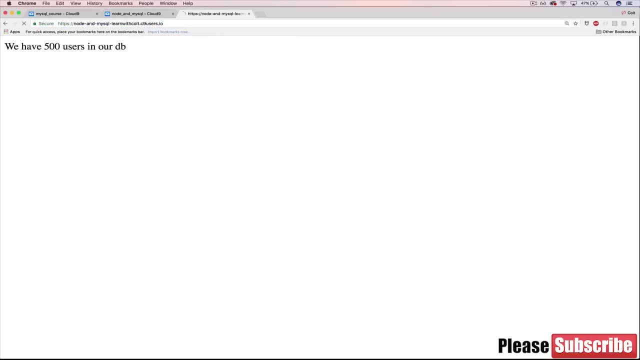 If it's an error, throw the error. Otherwise, select or isolate the count from the results. Then we do a res dot send. We have space count, space users in our database. Let's try it. And there we go. We have 500 users in our database. 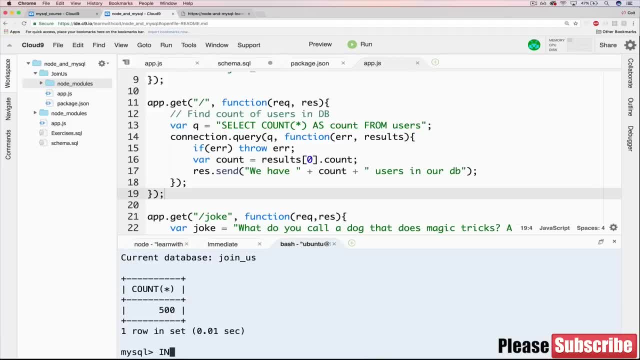 And to prove to you that it's working, let's go over here, Let's do an insert into users and we'll just do an email And we'll do something we haven't done. So an original here. Austin at Gmail dot com is still struggling with the originality there. 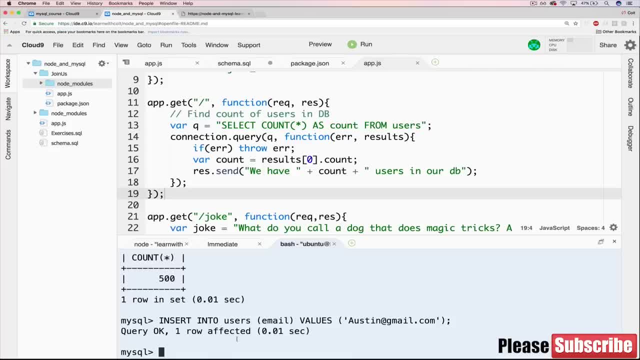 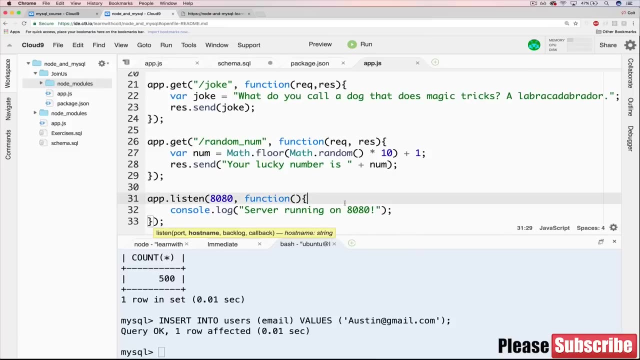 So we'll enter that single user, OK. so there now should be 501 and we can double check And it works. Note that we didn't have to restart the server or anything. that would kind of defeat the purpose if our data was only refreshed whenever the server restarted. 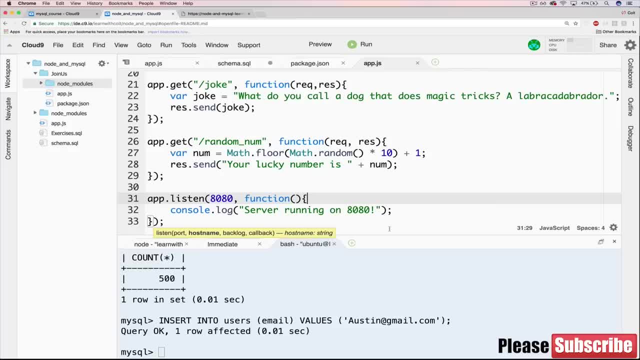 because we're going to have people interacting with this. When we set this app up and we finish it up, it will just be left running, you know, in perpetuity, until I don't know we have to fix something or I don't. 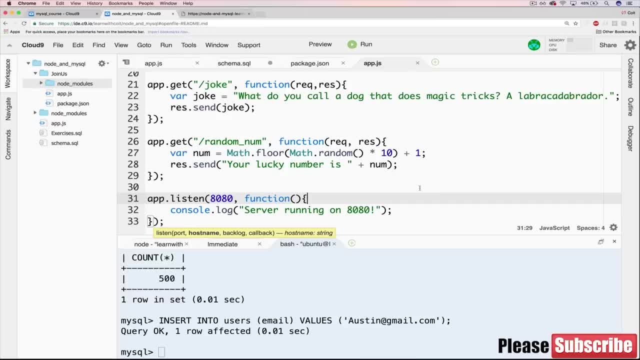 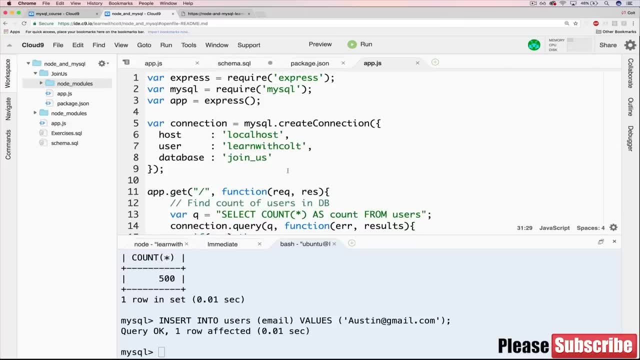 know we launch our startup app so it will be waiting, just running constantly. So our database will be changing all the time And it has a connection to that database. We can kind of check in with the database see how it's working. 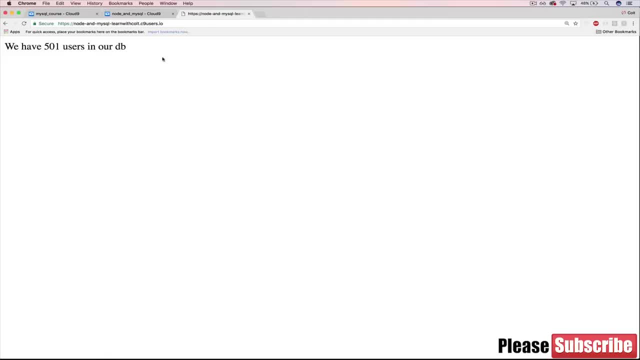 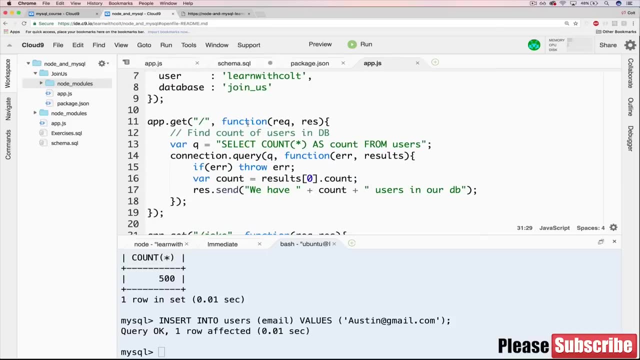 what's going on and get the results back and do something with them. So still very simple, But it's a start. So we're connecting with our database. The next thing that we'll need to focus on, which will take us a bit to get there- 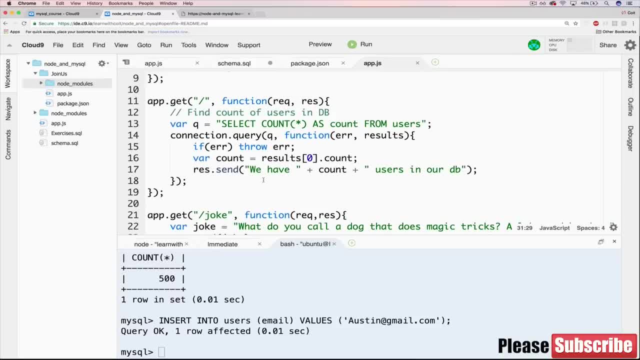 because we have to create the form and talk about HTML and a thing called EJS. But our next goal is to also run the insert query that will insert a new user in. But, like I said, to do that we have to set up the route that will. 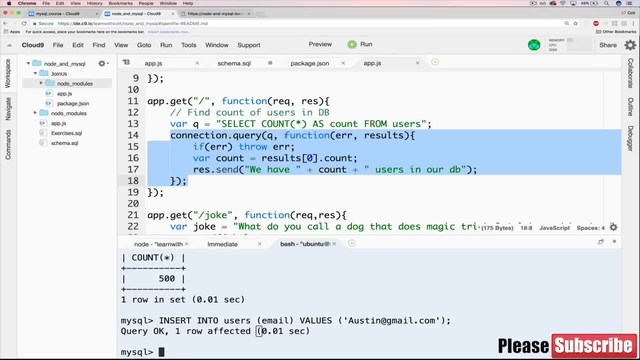 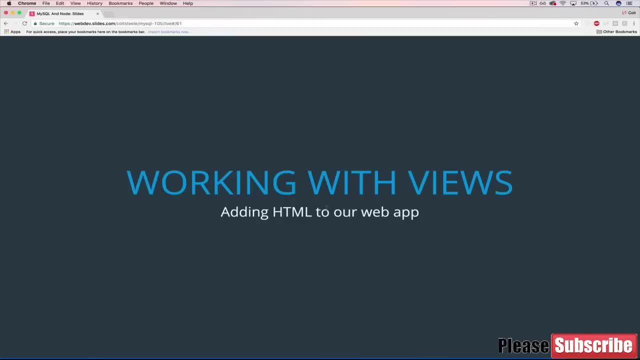 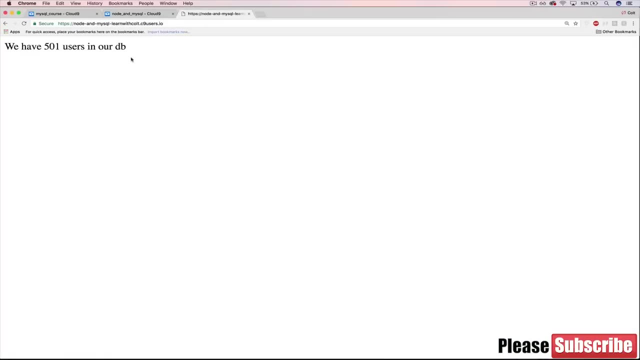 insert and we have to set up the form to actually do the insert for us. But that's where we're heading, OK, so now what we're going to focus on is actually getting HTML implemented with our Web application. So right now we're responding with these little ugly things of text like this: 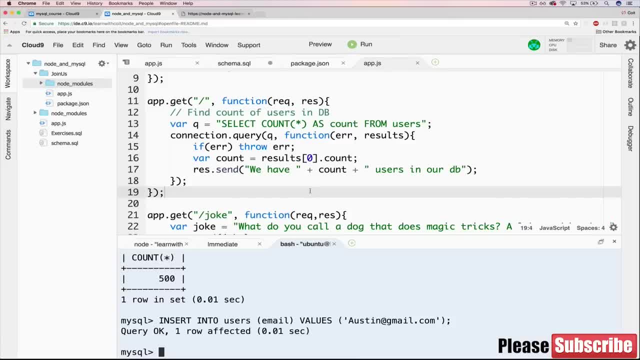 And before I go too much further, just another note. If you know HTML, great. If you don't know HTML, you'll just sort of have to hang on for the ride here. I'm sure you've heard of it, Well, I guess. hopefully I'm not assuming too much, but most you've come across HTML. 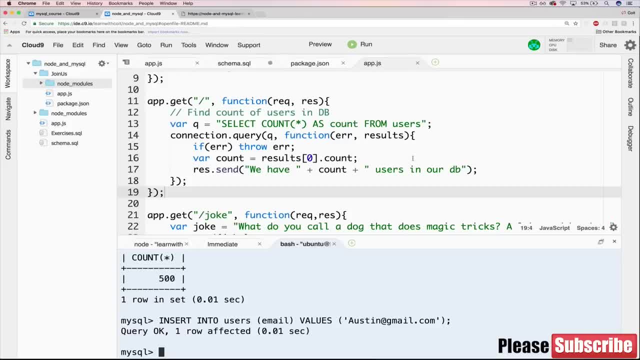 Every Web page to look at is built with HTML. behind the scenes, There is this markup language- It is dictating what elements go where, And then there's CSS- which we'll get to later- which makes it look pretty. So what we're going to do is focus on writing HTML so that we can have things. 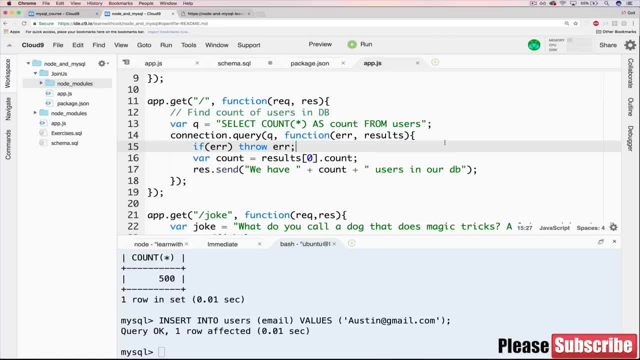 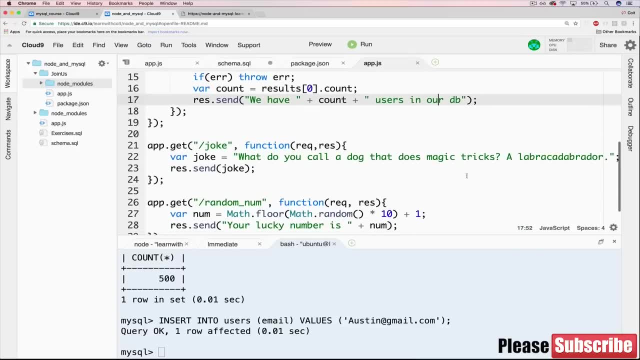 like a form and a button, or we can have large text, which is known as an H1. And we actually can do that right now in a really hacky way. So let's say, rather than just: well, let's do it for my joke. 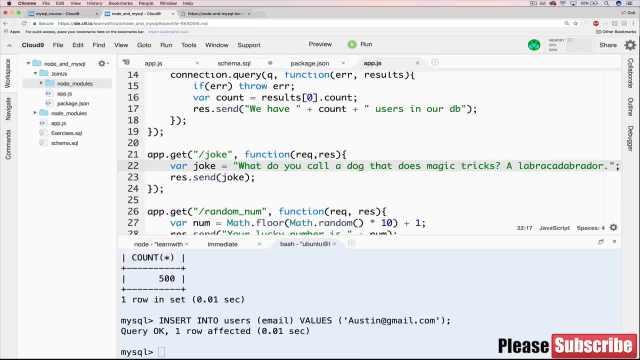 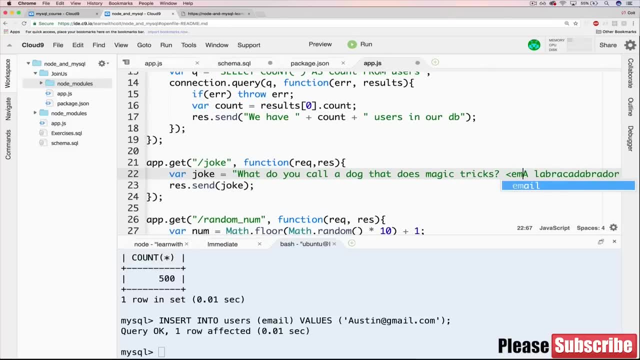 What I could do is make this joke, italicize part of it. So I'll say: what do you call a dog that does magic tricks? And I'll italicize the answer by putting around it the EM tag, which is how you make things. italicized. stands for emphasis. 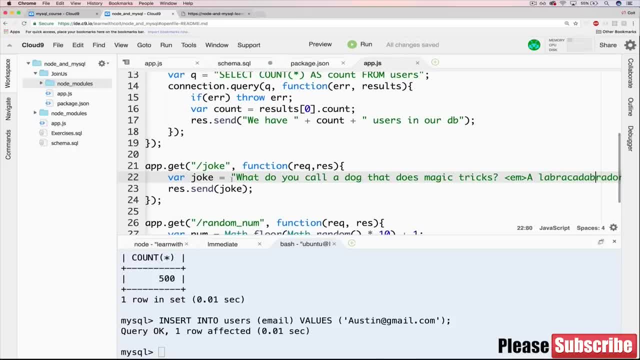 So if I just put HTML inside of this string- and actually I can make this bold too, so I'll do strong. First thing you should notice if you've ever written HTML, this is a horrible way to write it. instead of a single line like this: 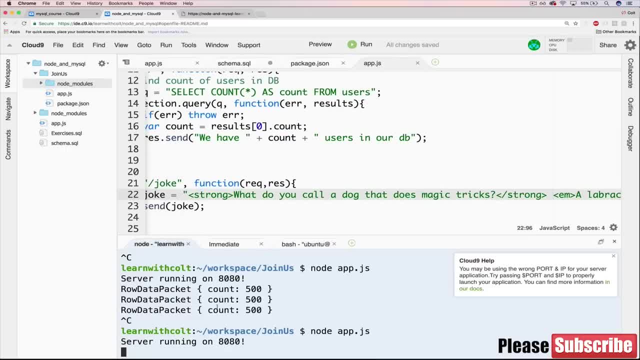 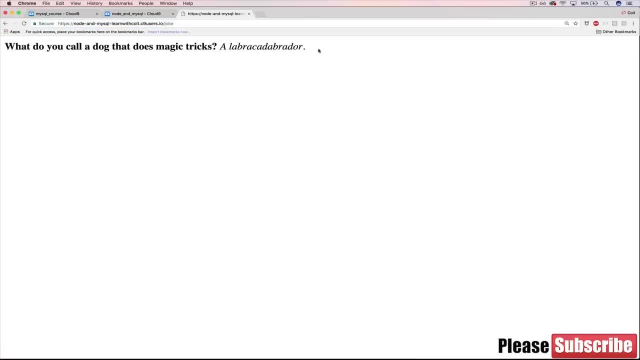 It's just not a good experience. So we're going to see how to get around that. But I'm more just showing you it's possible to have HTML in there. So if I go to slash joke you can see I'm getting HTML. that's being rendered properly. 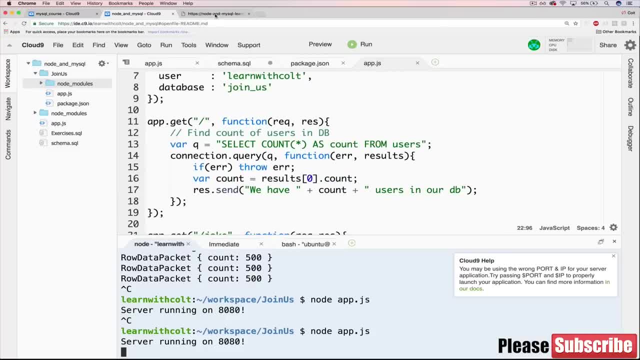 So if we wanted to get like a form on our homepage, which is what we want eventually by the end of this video we could put all the HTML to make a form inside of this string. But it's going to be significantly longer than this. 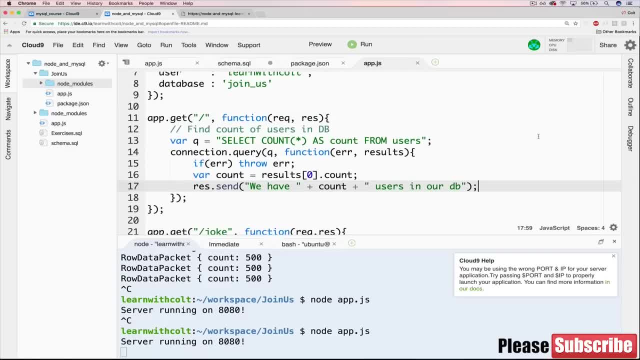 So we're not going to do that, And there's a bunch of reasons why. the main one is that it's a pain, But it's also hard to change things And it doesn't really allow us to style it with CSS when we get there. 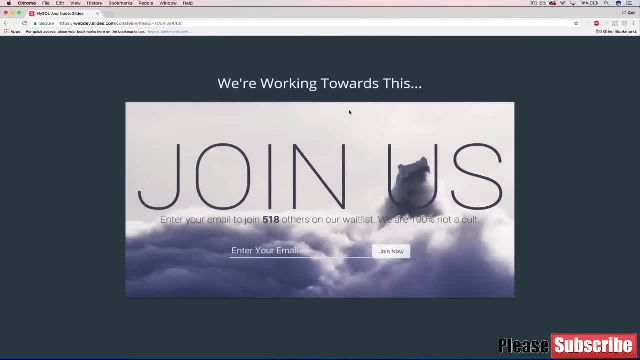 So, to jog your memory, this is what we're working towards. This is what our app will look like. We have a big background photo of a beautiful mountain in Argentina. Then we've got join us. big text, different font, different color. 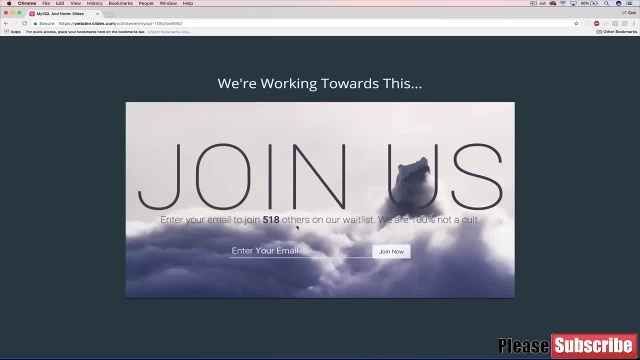 Then we've got this other text: Enter your email to join 500 or whatever the number of users is Others on our wait list? we are 100 percent, not a cult. And then we have a form with a single item in it. 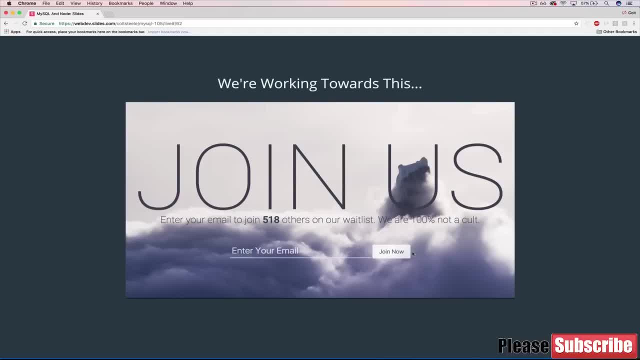 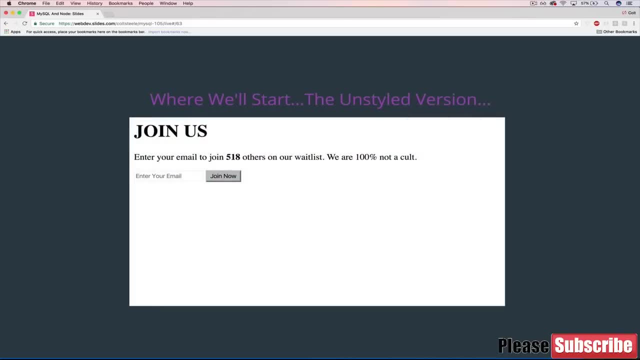 A single field, a text field and then a button that will submit the form. But if we strip away all the pretty styling, all the makeup or paint on top, This is what it looks like. This is, you know, the bare bones of it. 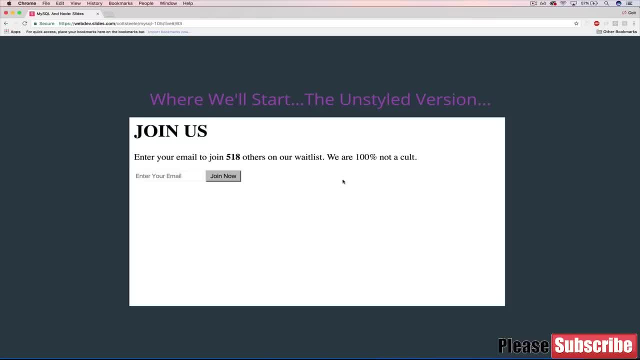 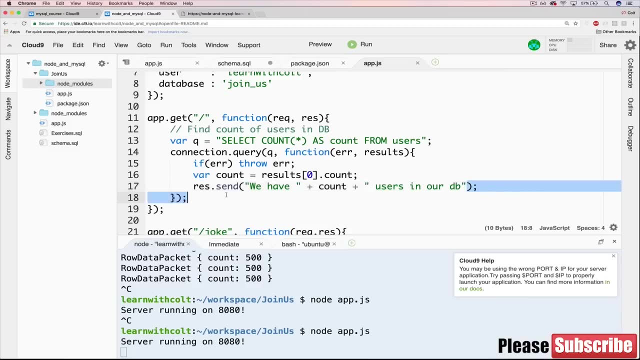 So this is what we'll get to by the end of this video, So this will be our home page. We are going to replace the content here, The single string, with this, and to do it, there's a couple of steps we have to take. 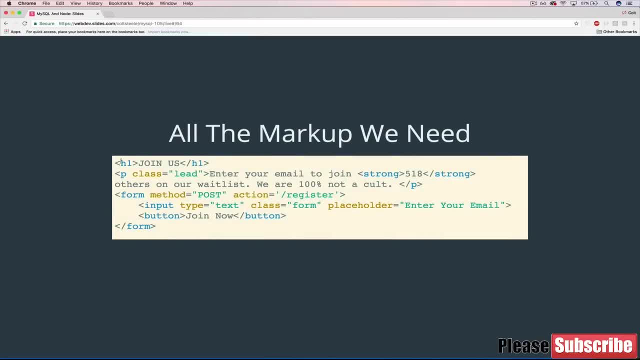 So here is the HTML itself. If you don't want to type it, this is the HTML we need. We've got an H1 that says join us. We got a paragraph. We'll come back to this class. We don't need that actually right now. 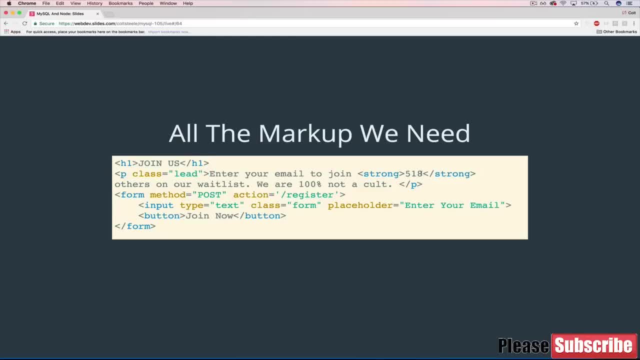 But then we've got enter email to join strong, which is the bold around 518.. Then we've got a form which we'll also come back to. So I'm just showing you. this is all we need to actually make the HTML the correct. 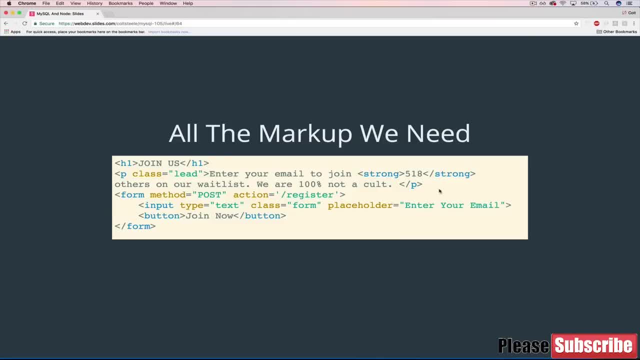 HTML to make that page. Now, how do we actually get this to be sent back? What we want Is, in this route, when you go to slash, basically give the user this. We can't just make that a single string. So what we do is use something called EJS, and you have to bear with me here. 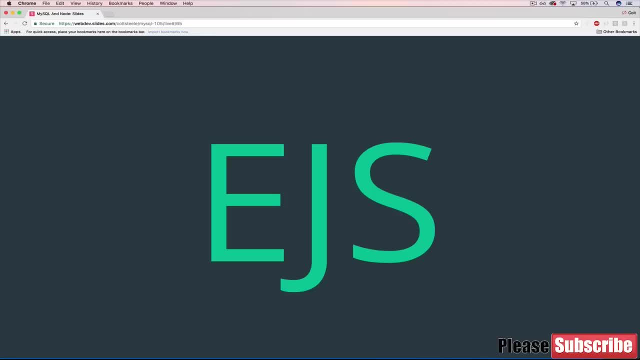 There's a couple of steps you have to go over And if you're new to web development this will be a bit intimidating Possibly. it's probably a terrible thing for a teacher to say, but just hang in there. Just know that we're going somewhere and some of the steps along the way may. 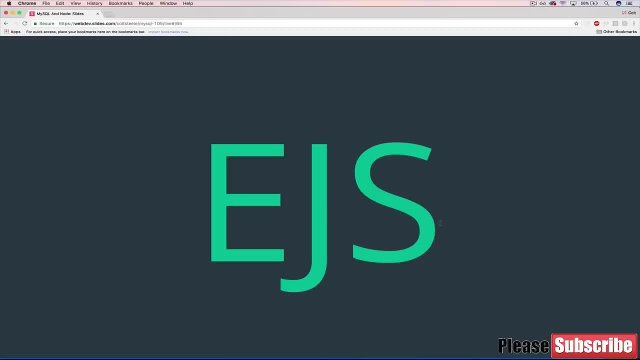 be confusing, but once we get there it won't be too bad. So EJS is what's known As a templating language, stands for embedded JavaScript. It's an alternative to writing just plain HTML. It allows us to add in variable values and code logic. 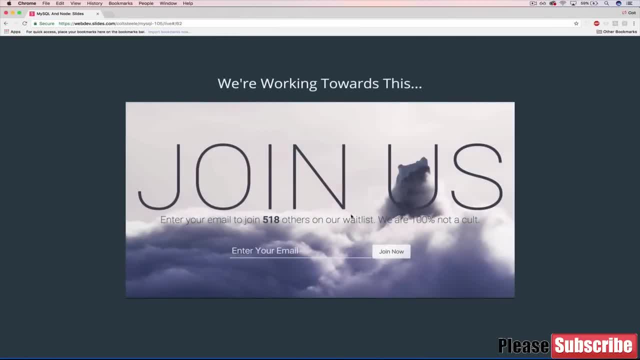 So this is where's that slide. Go back here. This is HTML, But this right here is not always five hundred and eighteen, So we couldn't do that in a normal HTML file. We would want to be able to say: OK, this is HTML. 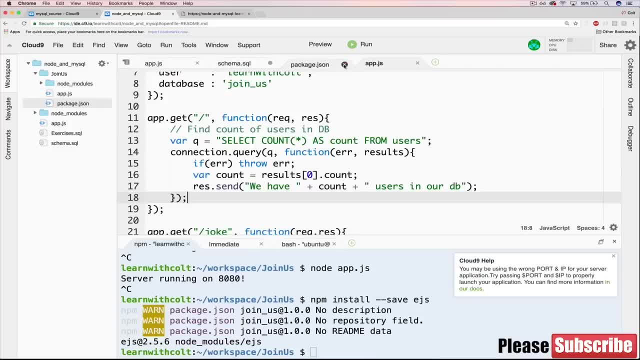 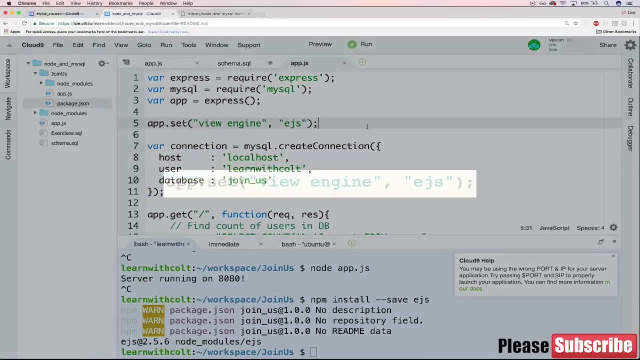 But right here in that strong tag, in the bold area, there's a variable. but you can't do a variable in regular HTML, So that's what we're going to use EJS for. It stands for embedded JavaScript. It's just HTML that allows you to embed JavaScript inside of it. 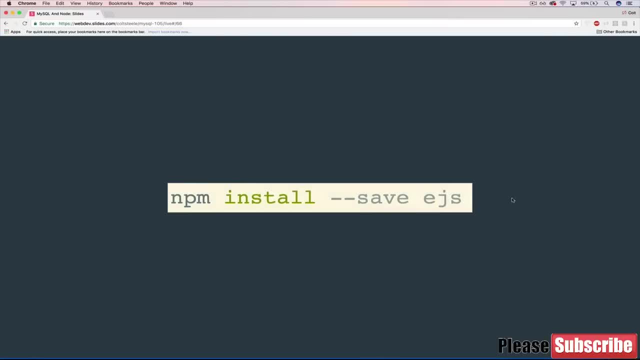 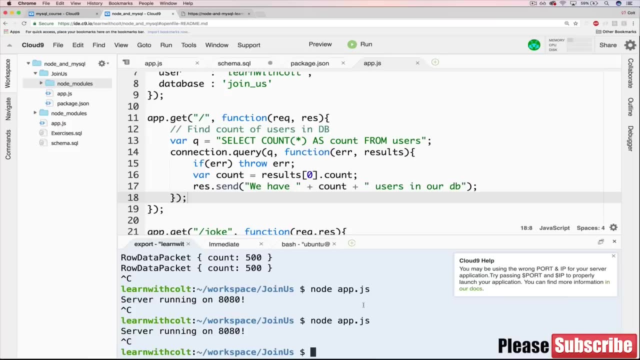 So we'll see how to do that in a moment. But the first thing we have to do npm install dash, dash, save EJS. This is you know. you should know by now, hopefully, that this is going to tell our app and our packagejson that we want. 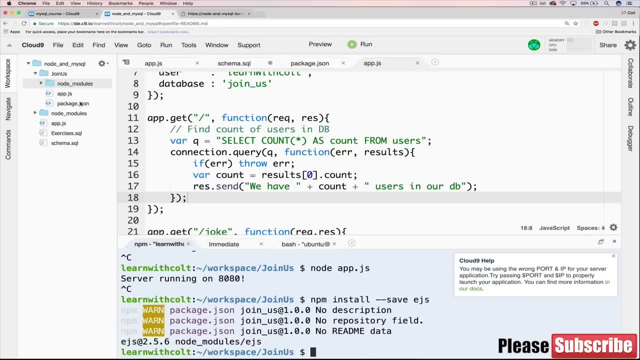 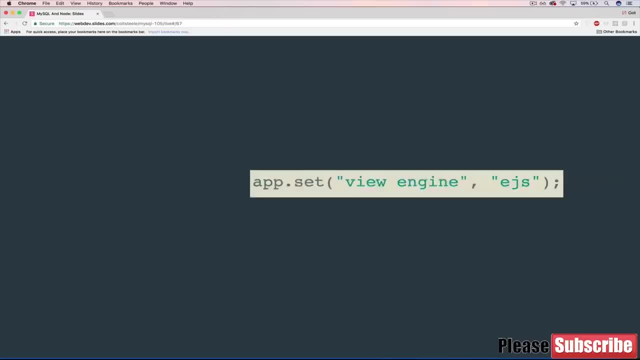 EJS installed and it should install it and save a record to packagejson, which you can see. now we have EJS there. That's our first step. Then we're going to do something else. This is configuring our express application appset view engine comma EJS. 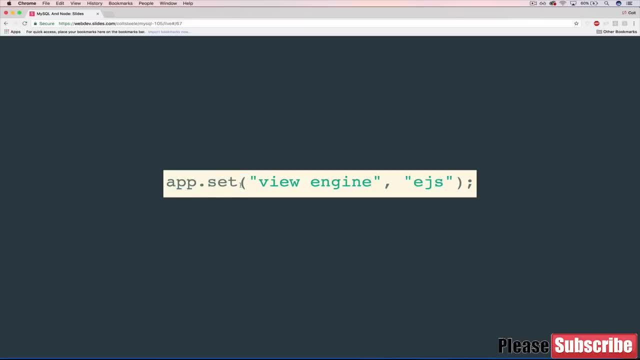 So appset is a method that allows us to set certain settings in our app. View engine is the most common one to change. There are other templating engines. There's things like Jade, which is a common one, Hamel- there's other languages. 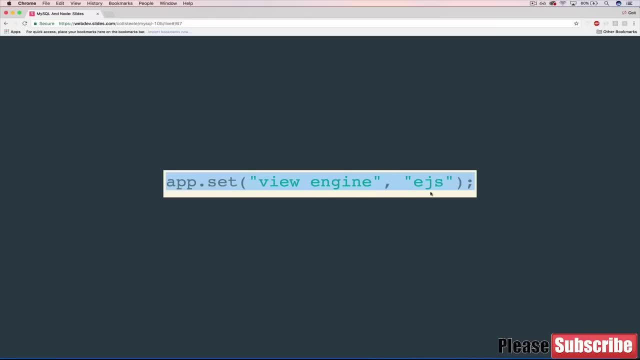 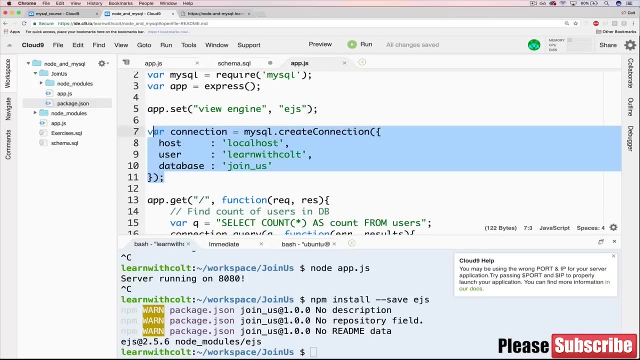 So basically they are similar analogs to EJS. Okay, so we'll go do it at the top. It's a traditional place to do it. just like we're setting up our connection up here, It makes sense to set and to configure application wide things up top. 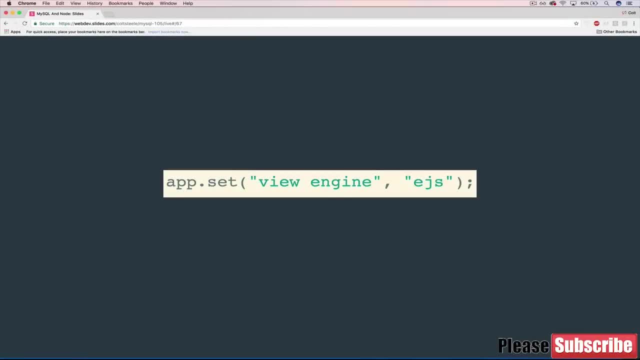 So we'll do that, And then the next step is: okay, where do we actually start writing these files? And to show you that I'm actually going to work backwards, So the line that will be running in our route that will actually render a file is res dot- render some string in our case. 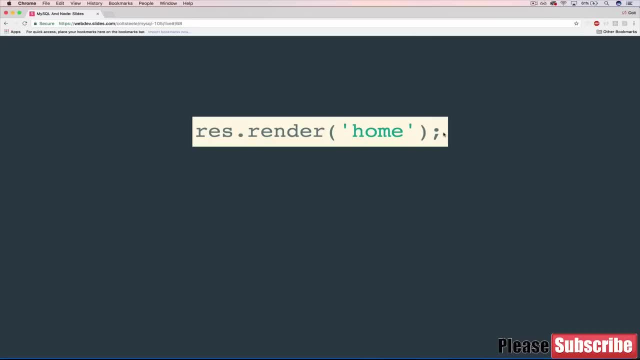 home and the process that will happen behind the scenes that Express doesn't really show you or tell you about is it will automatically look for a directory called views. That's a standardized name. So it's going to look for a directory called views. You can change that if you wanted to, but we're not going to. 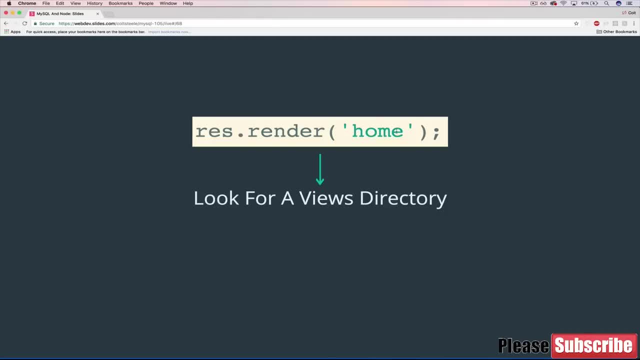 And inside that directory it's going to look for a file called home dot, whatever the view engine we said, which is EJS in our case. So it's going to look for home dot EJS in that views directory. So what that means is we need to create a views directory and then we need to create 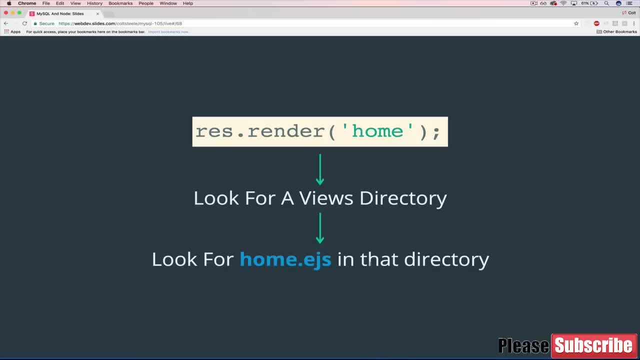 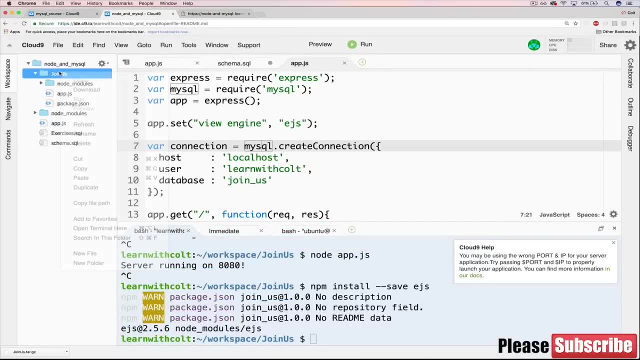 a file. we'll call it home, but you could call it landing page dot EJS or root dot EJS. Whatever it is, you just need to remember the name. So let's do that now. We'll do right click or you could do make directory. 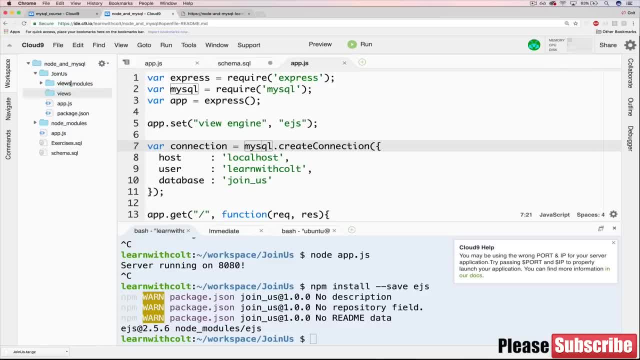 If you're more comfortable with a terminal, new folder views inside of there. we'll make a single file which we will call home dot EJS. Again, you could call it whatever, as long as it ends in EJS And you remember what you call it. 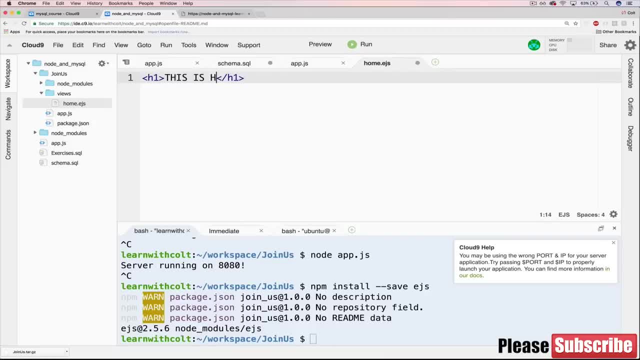 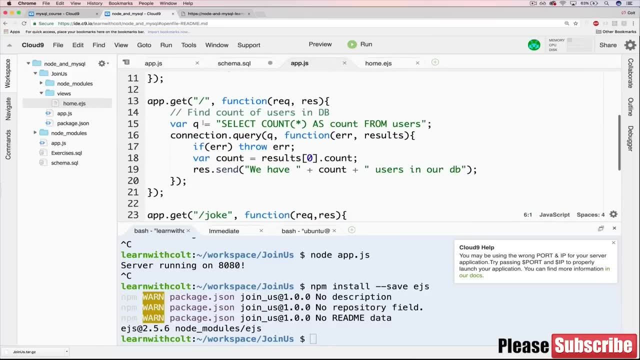 And we'll start with a single H1.. We'll just say this is HTML and save it. Then we go to our app JS and let's just work with our route route rather than sending this dot send. We have count. We're no longer working with res dot send. 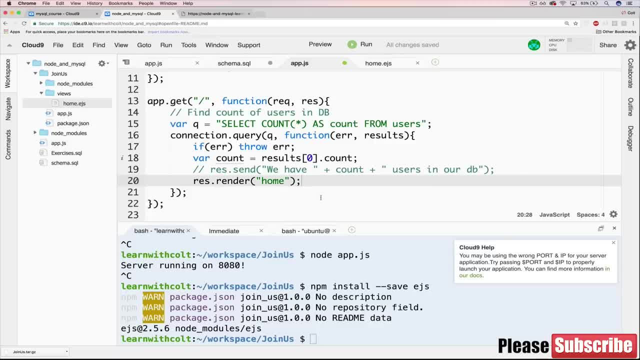 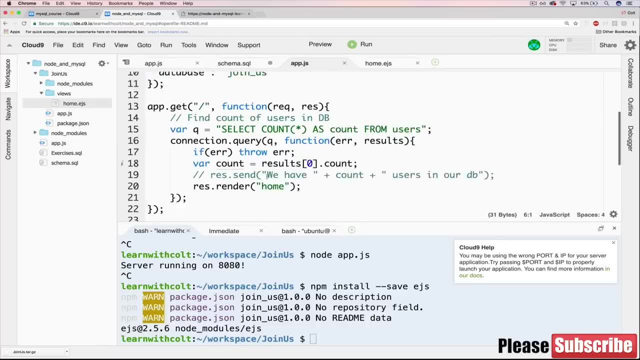 We have a res dot render home. Just- I'm going to be a broken record, but it's looking for home dot EJS, because we added this view engine is EJS and it's looking in views by default, So we need to make sure we have that file. 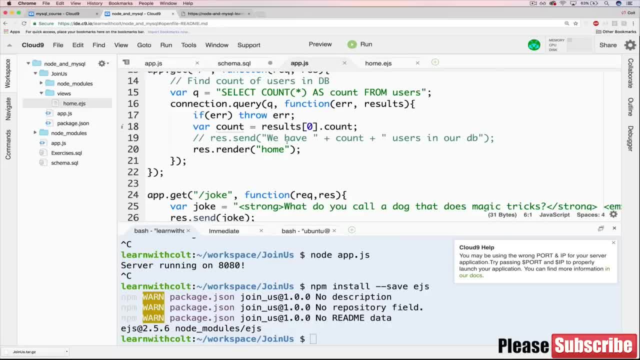 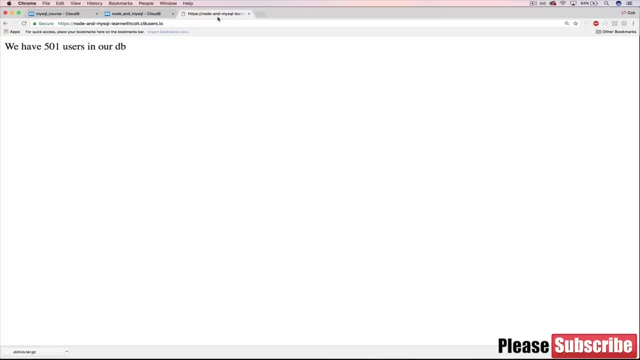 It's going to take the content to this file and send it all back. rather than a single line, we can write our code now in a separate file, So let's see if it works. Start our app. Let's try going to the home page. 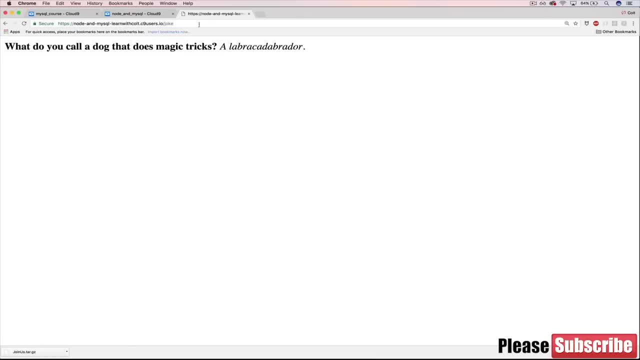 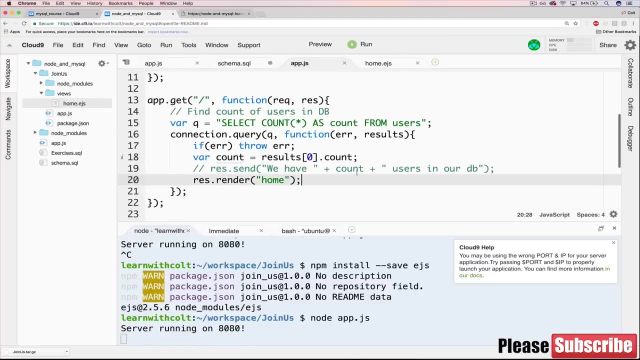 There we go. This is HTML Our other pages still have. Well, this one is HTML, but it's not coming from a separate file. OK, so then what we can do next is I'll just show you. You could use res dot render home. 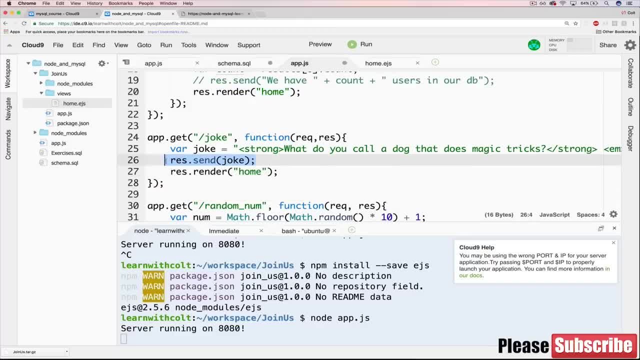 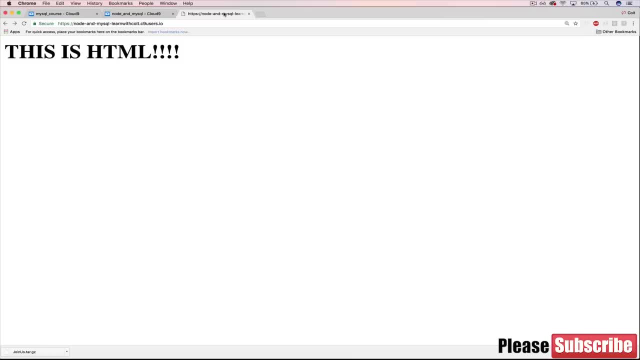 You can send the same file in all of these. instead of res dot send, You can reuse files in different routes, It doesn't matter. So here we have the same thing for joke. So now, if I go to slash joke as well, I get the exact same thing. 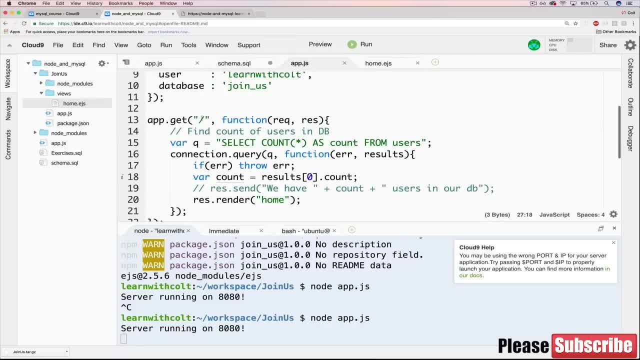 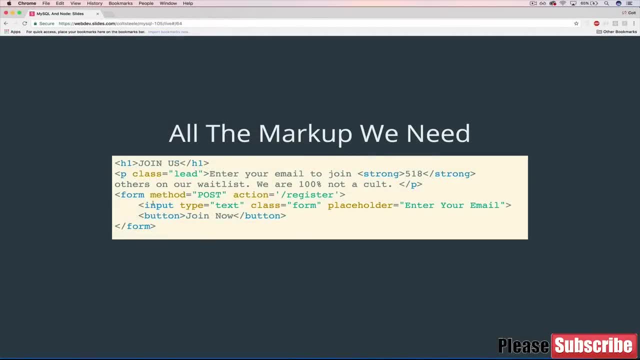 OK, so these don't care about what they're called. The name of this has nothing to do with the route, although it should. if you're just following best practices, I'll get rid of that. So now let's just copy the HTML that I 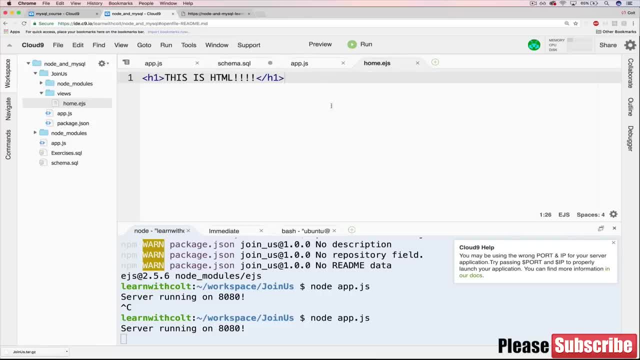 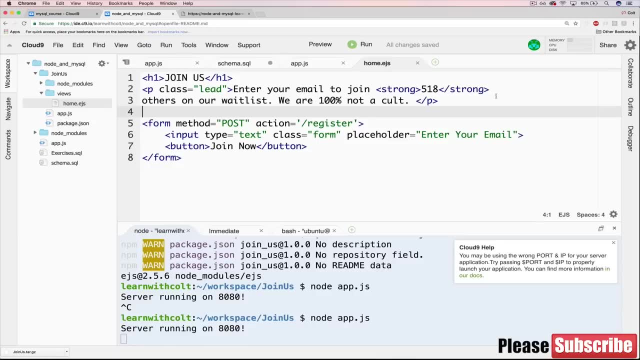 provided here so that we don't have to type it all ourselves. So in home dot EJS. I'm just going to paste this in. We'll go over what some of this is, in particular the form we haven't talked about, but let's just get this in here. 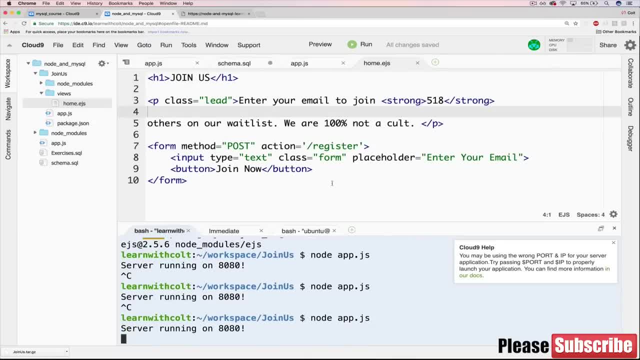 And see how it works. So we have to save the file. Now we get our form, So we have join us, which is our H one, which is what we started with. Then we have a paragraph again. Don't worry about the class at all for now. 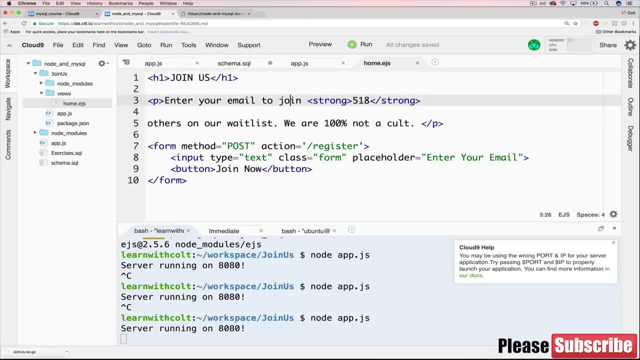 You can actually just get rid of that. if you want Just focus on keeping it simple, Then we've got enter your email to join instead the paragraph. All of this is in the paragraph. There we go. 518 is hard coded for now. 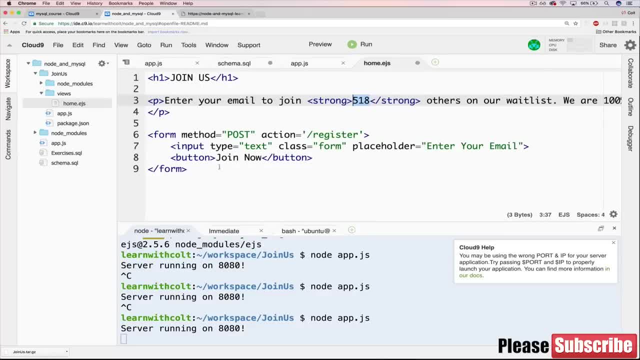 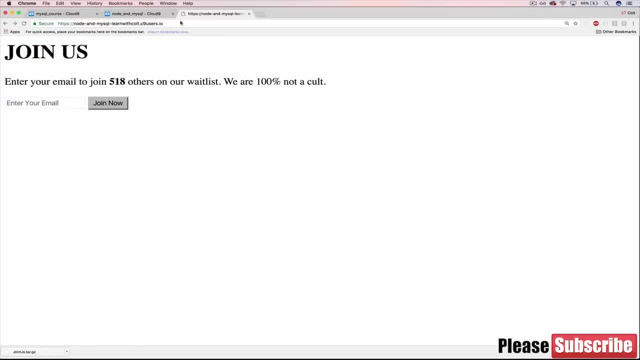 We're about to Replace that. We are 100 percent, not a cult. And then we've got this form, which we're just going to ignore for now, except know that there's a text input and a button which we get at all looks good. 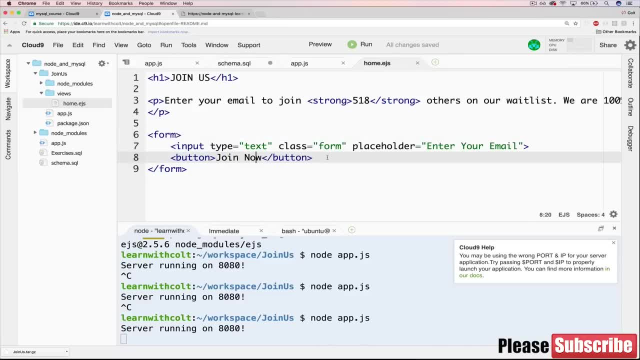 And, in fact, we can clear out that form and just leave it like this to start. OK, so now what we want to do is figure out how we get our data in here, because right now, this is just plain HTML. There's no use for this stuff that I was talking about. 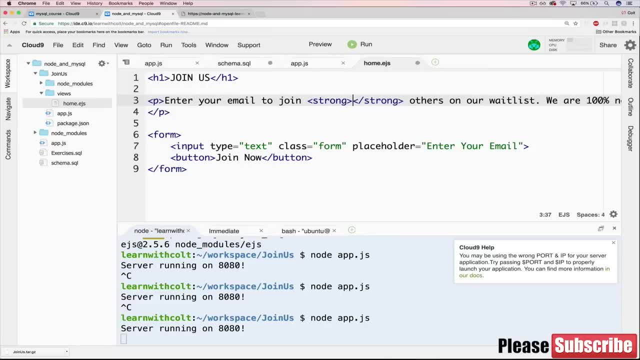 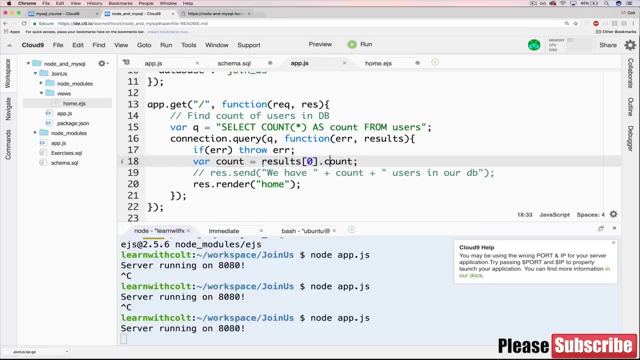 But the whole point is that we want this to be 519,, 520,, 499,, 10,000, whatever. the result of this is, whatever count is. But how do I get count this variable over here? What we do is, after res, dot, render, we can pass a comma and pass a JavaScript. 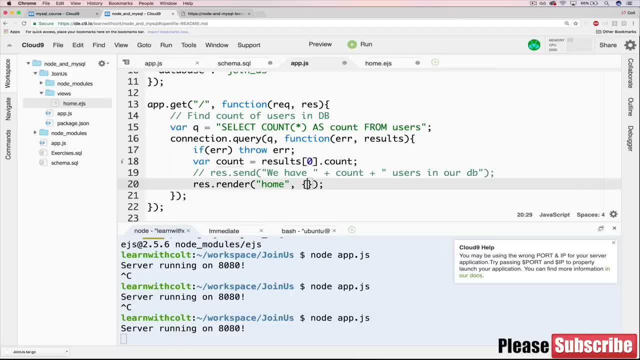 object and I'm allowed to pass data through. So what we want to send is count, But first I have to give it a name. So typically you'll see something like this: count, count. So rather than that I'll do, data is count. 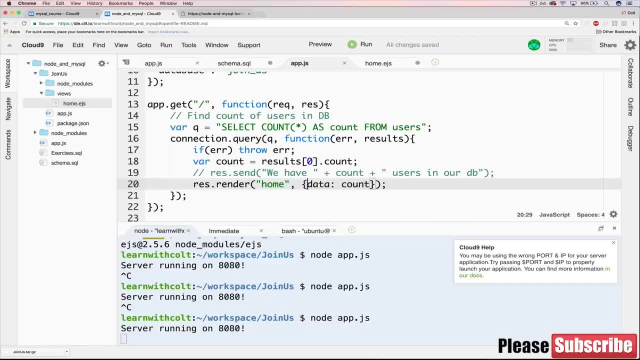 I'm going to change it later, but just to show you they're distinct. So what this does now is it says: OK, take count, whatever it is, which last time we counted was 501,, send that to this template And give it the name of data. basically put it in an object under the key of data. 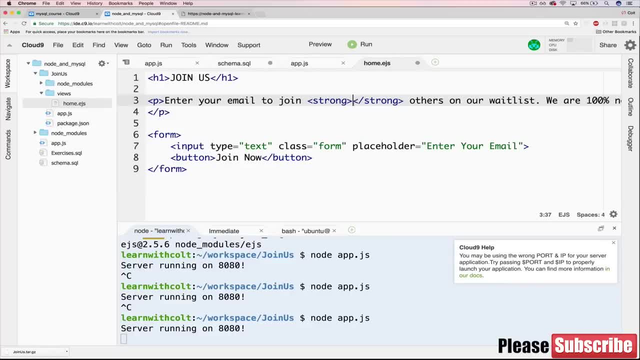 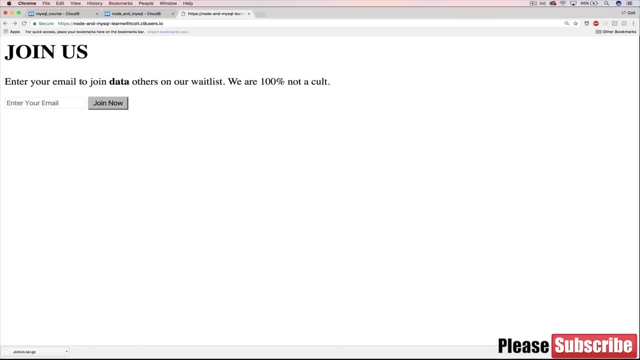 So inside of here if I refer to data, it will be referring to whatever count was. The problem is I can't just say data. If I just do that and refresh, we just get enter your email to join data. Others on our wait list. 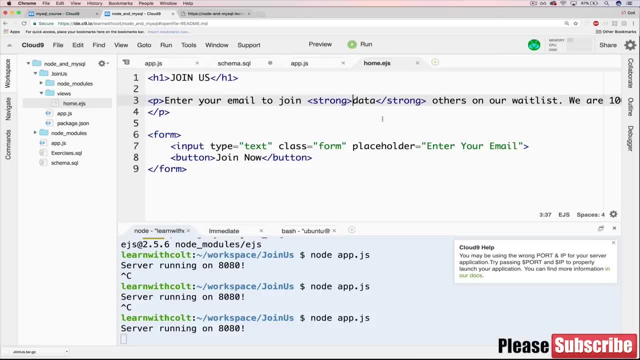 So I need a way of saying, hey, this is not, this is not HTML, This is special, This is code And the way we do it. it's weird if you've never seen it before. It looks like this: So we have brackets, just like we would with HTML, the angle brackets, but then percent. 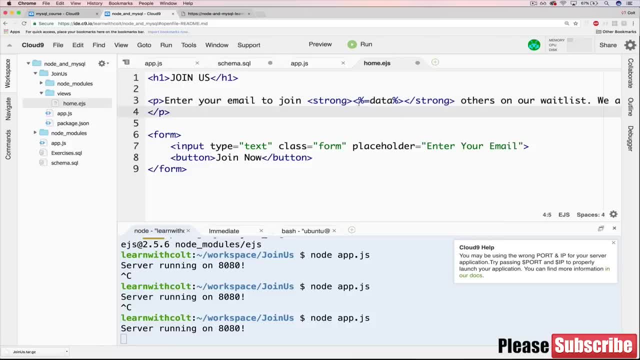 equals And then percent on the closing side, And this is basically a signifier that says this is not HTML. Whatever is in here is going to return a value that we want to put in the HTML. So if data is equal to 500, it will be replaced with 500. 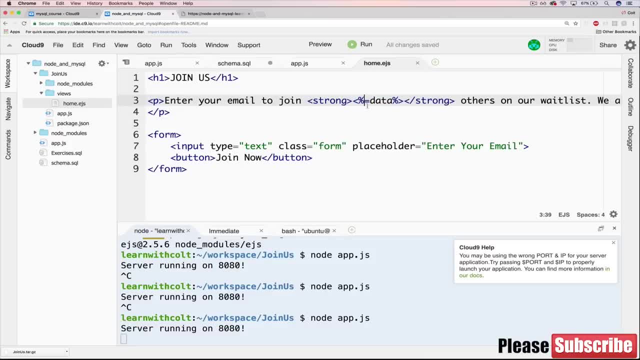 If it's equal to 12, it will be replaced with 12.. Kind of a lot to take in. as I was saying, there's a lot of moving pieces here. Unfortunately, we don't have- well, we don't really have time. 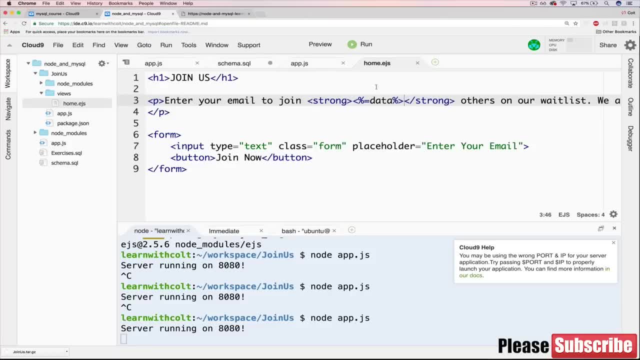 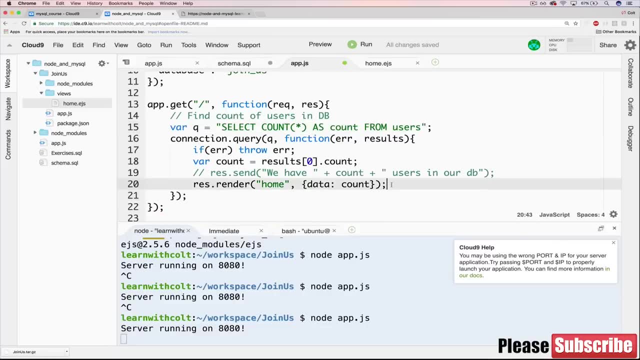 I guess we could. we could have time, but the course isn't on EJS, it's not on web development. This is just a vehicle to showing you how to make something OK, so data will be count whatever is coming through there. 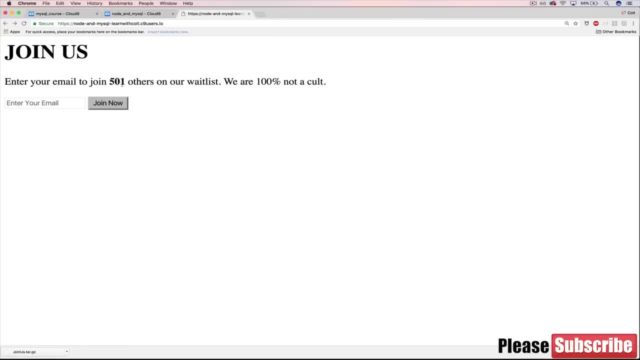 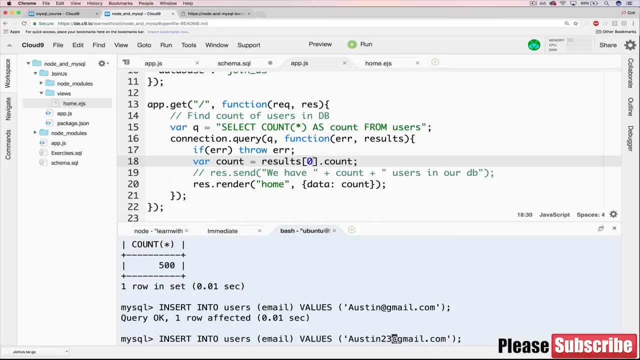 Let's try it, And we've got 501.. And of course, we could insert one more user very quickly. Let's do Austin 234.. Refresh our page Now, it's 502.. So we've accomplished our goal. If you feel comfortable with how it's. 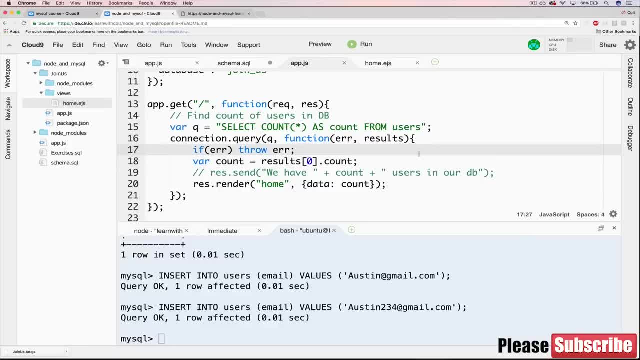 working. go ahead, stop. move on to the next video. If you have a couple of questions, though, I'm going to go through the process again. I'm not going to recreate it, but I'm going to step through what's happening. 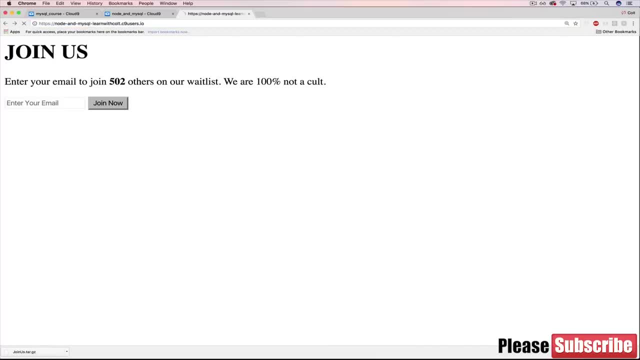 So we'll start with this app: dot get slash. that's activating the route. when I go to this URL, We still have our slash joke. for instance, We're talking about the route route. When I hit that route, first thing that happens is this code runs: 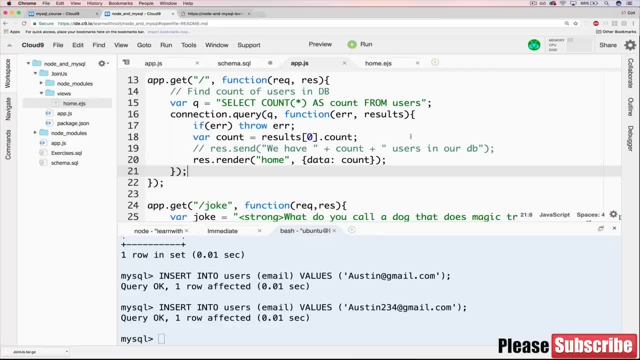 which the end result is. It figures out how many users are in our database. It's running this code in our database: Select count star as count from users. That's coming back stored in results Inside of results. we're finding it. 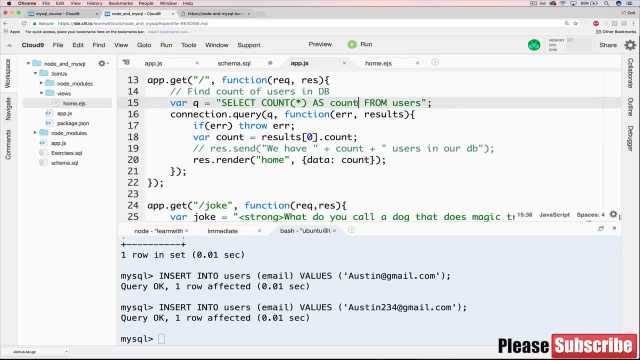 The reason it's stored under dot count is because of this as: So if I called this counter, then this needs to be dot counter. OK, so then we're storing that in a variable called count, So this has something like Five hundred and one in it. 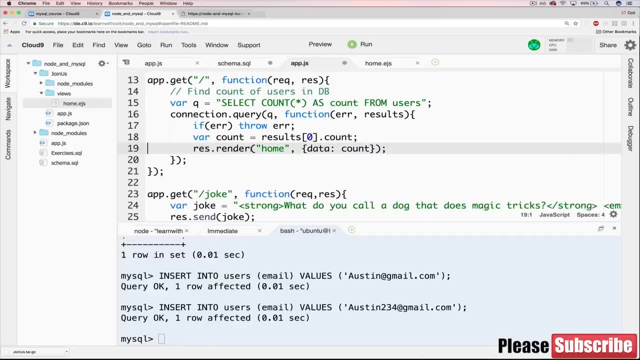 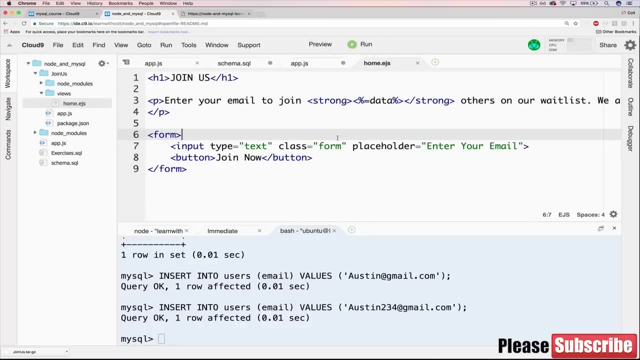 Then what we're doing can get rid of this line now Is we are rendering the home dot EJS file, which is automatically looked for in the views directory, which is right here. We have a bunch of HTML in here, some of which we haven't talked about yet. 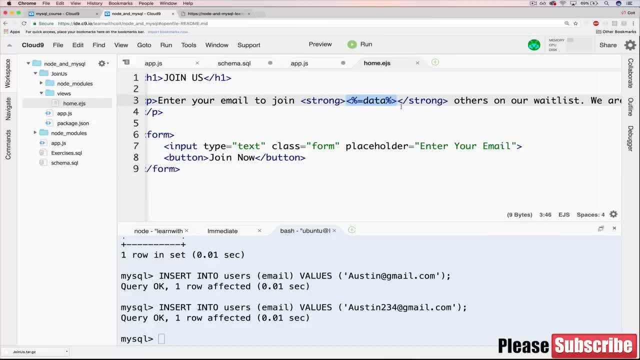 But then we have this one variable with this very weird syntax we haven't seen before. This is our way of saying: hey, this is not HTML, This is a Special value. We can put JavaScript in here. and just to show you a couple other things: 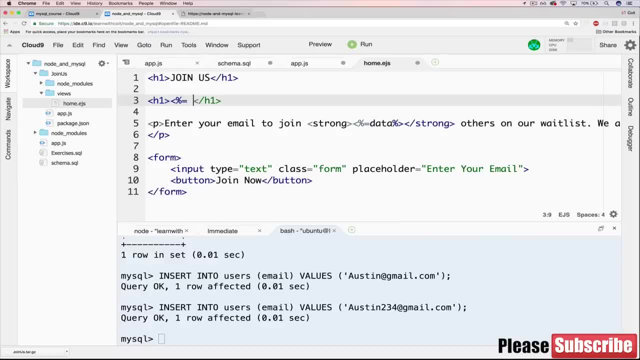 I'll do another H1 and then our funky bracket thing again, And I can actually just do simple math in here. Let's do something like four times ninety eight. This will run as JavaScript. Whatever the result is- I'm terrible at mental math- will be printed there. 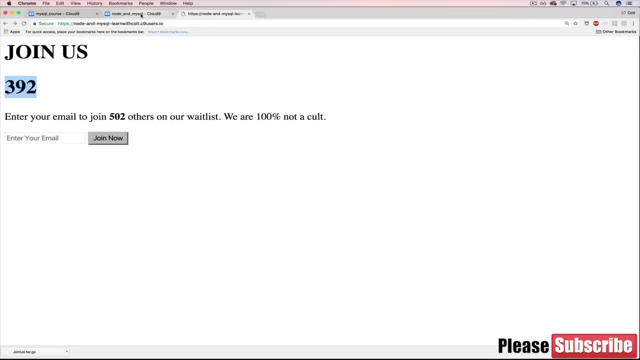 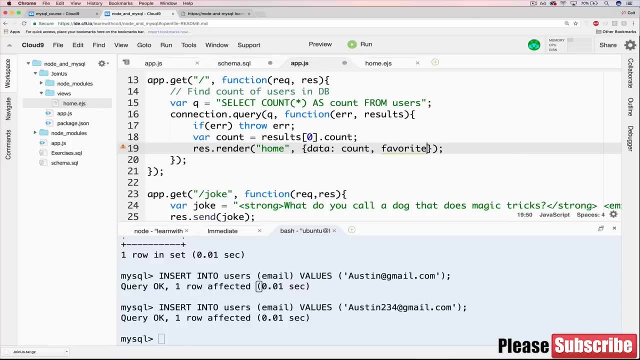 So if we refresh our page, we get three ninety two, And we could also pass in another piece of data like favorite color, And I'll just say it is purple, which is true, My favorite color, highly underrated. Pass that in over here. 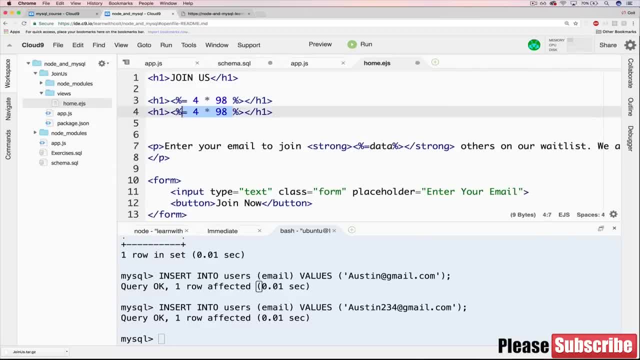 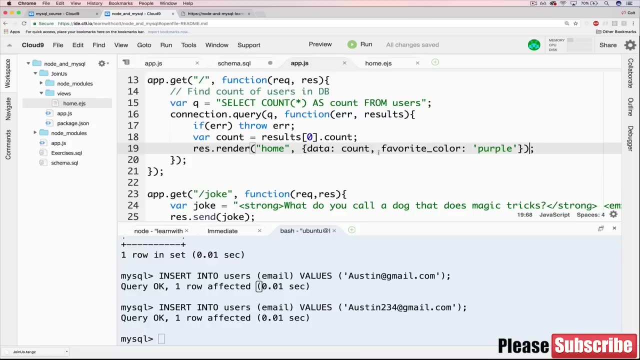 I can refer to favorite color. Why we would do this, Well, that's another question, but I'm just showing you that, Oh boy, Here we go. Favorite underscore color. We Have access to whatever we pass in here. 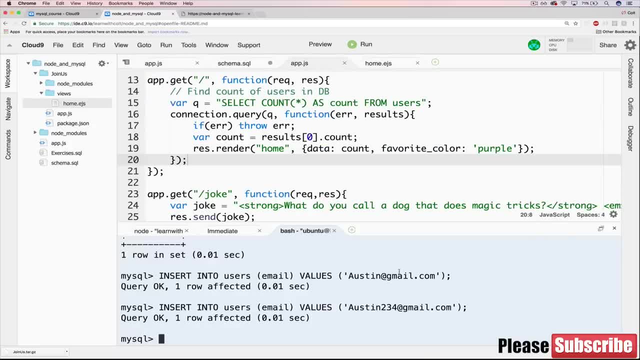 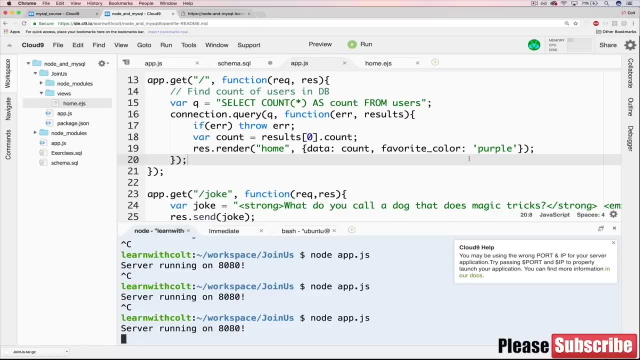 So favorite color is a string: purple. I will need to restart the server if we are changing our app JS file. Now we get purple, It's coming through. So the only difference is that data right here is not something we're coding in ourselves are not hard coding. 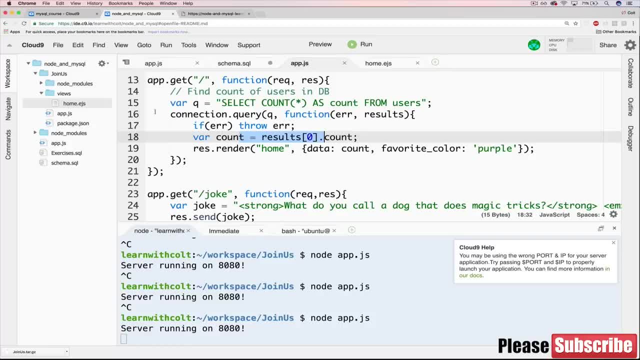 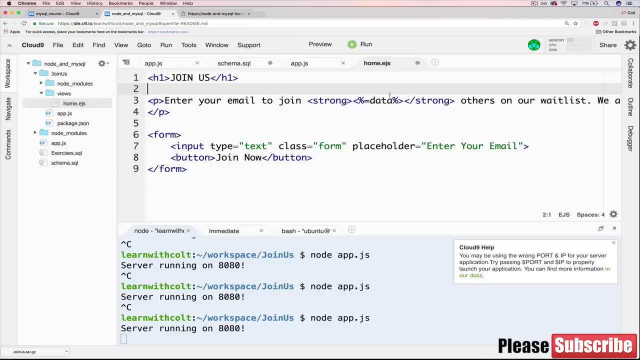 And it's coming from the database, From all this work running the query and then basically extracting the data out, saving it into the count variable, And the last thing I'll do is change this to be count, because data is just a bad to bad name for a variable. Everything is data. 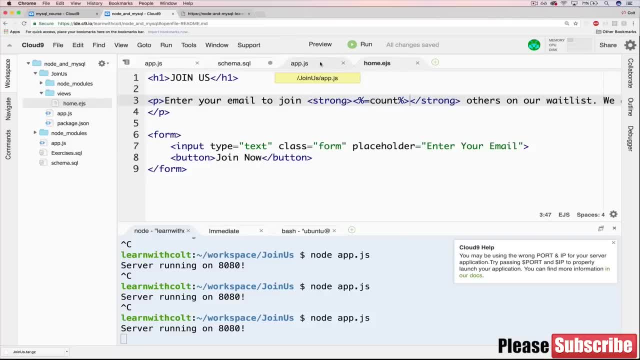 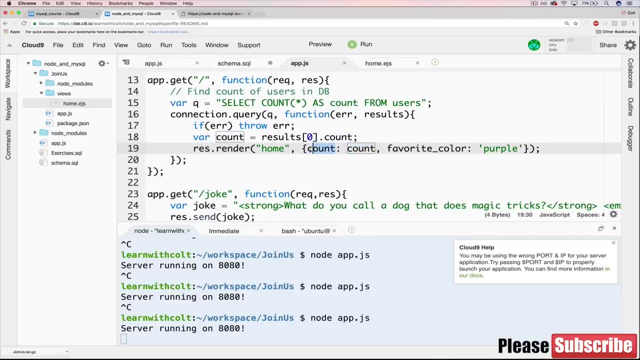 But the reason I called it data again was just to kind of show you that there's a difference. it can be confusing at first if you see count, count, which one is which? This is the value we're passing and this is the label for it. 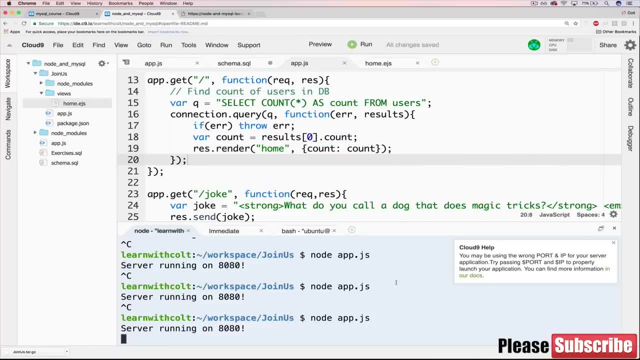 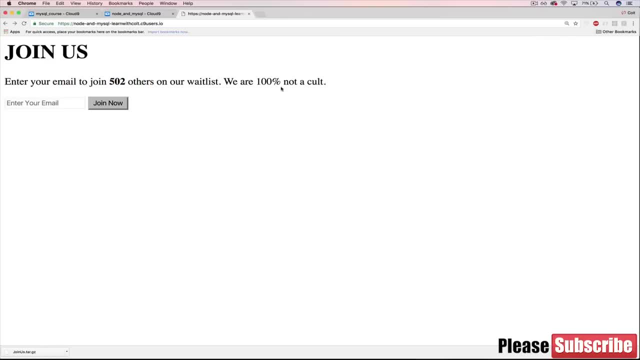 This is the key, OK, so let's just make sure it's still working. Refresh. Enter your email to join 502 others on our waitlist. We are 100 percent, not a cult Perfect. We're done, OK, so picking up where we left off. 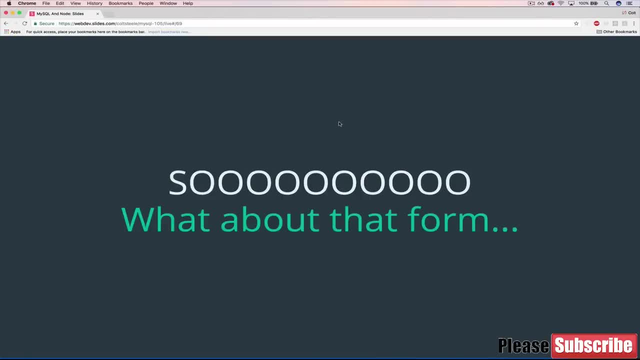 If you remember, in the last video where we got the HTML up and running the JS file, I said: ignore the form for now. we're coming back to that. Well, now is the video where we're going to get that form working, And it involves a couple of new concepts. 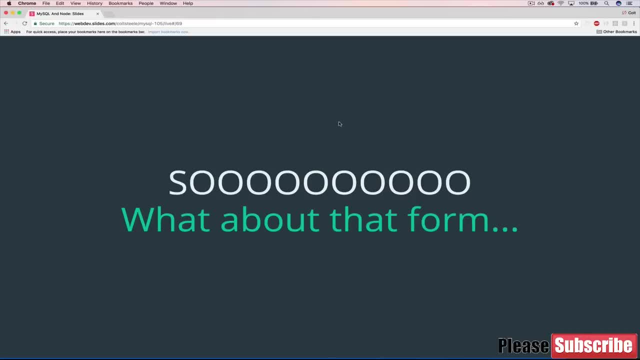 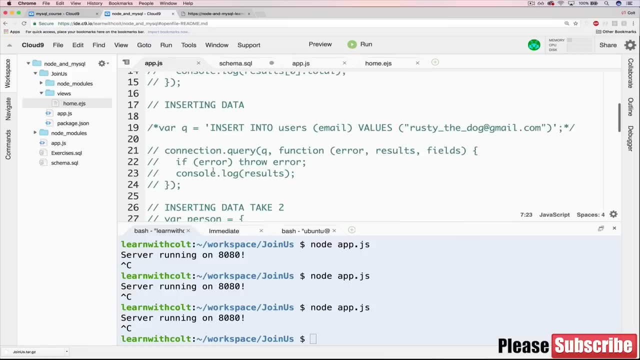 So hang in there. The MySQL part is the same. We've already seen how to insert. Let's go back to this early. Where is it? Here we go. We've seen how to insert a single file. We inserted this single rusty the dog. 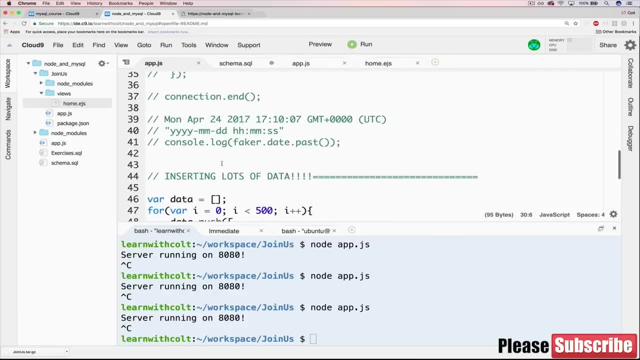 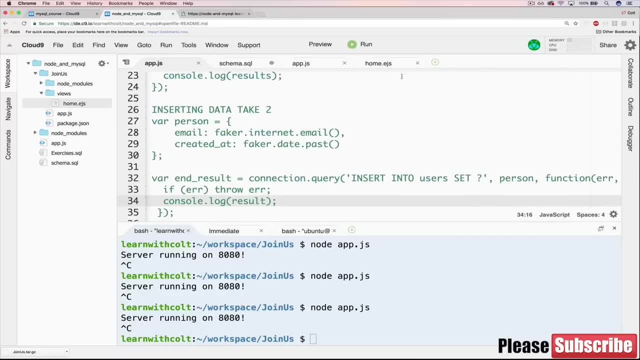 We also saw how to do it with this object syntax, And then we saw how to do a bulk insert with a lot of them which we don't need to worry about. So we've seen how to do this. Now we need to figure out a couple of things. 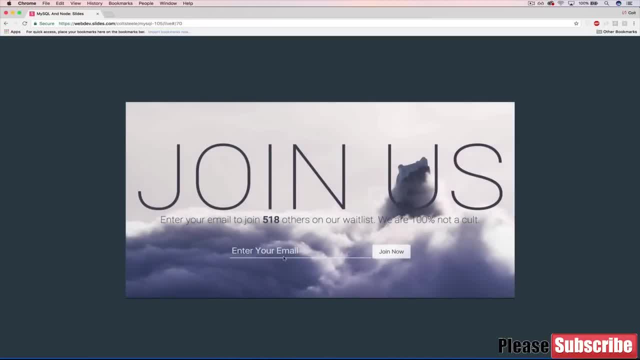 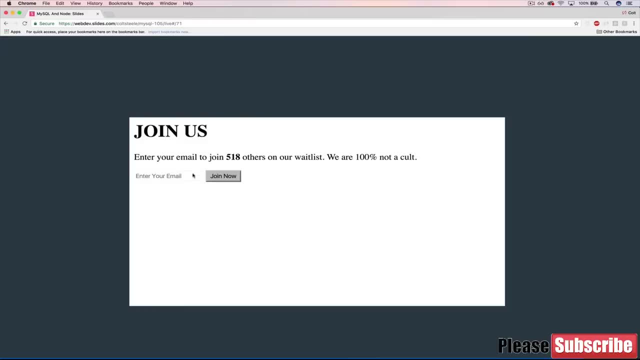 One: how do we get the data from the form, This form here unstyled. So this form, user types their email and it's joined. Now, First of all, where do they send that request to? We need to figure that out. 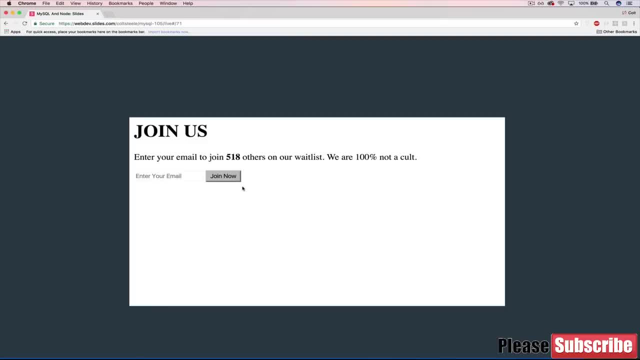 And maybe you guessed this. We need to define a route for that, But there's a slight difference in that route, which I'll get to in a second, because there's another problem, which is: how does that data from the form get there? 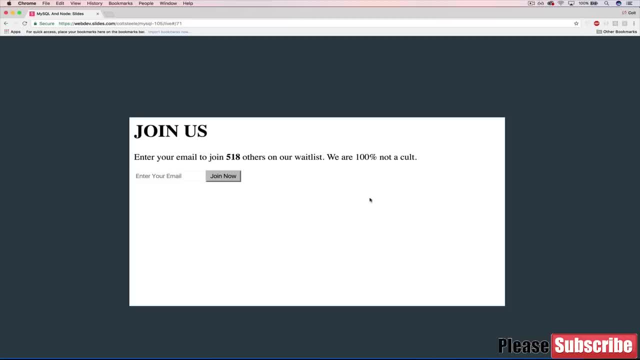 Well, what we want to do is use what's known as a post route, So there are different types of requests. I briefly touched on this: get and post request. This is not, of course, an HTTP, So you kind of just have to take me at my word here that we need to use a post request. 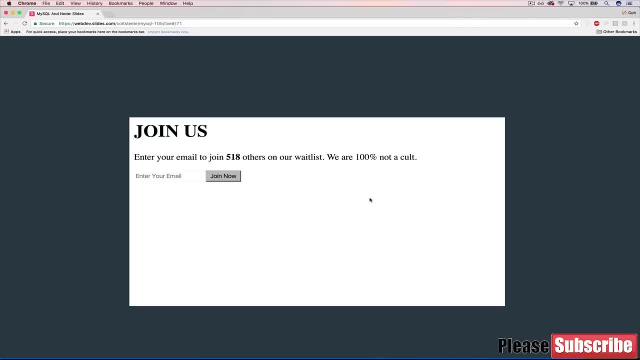 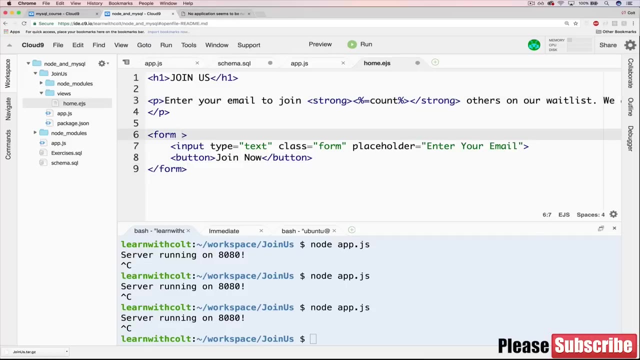 because it allows us to send data with the request. The form will automatically take the data from here and send it as a post request to the destination that we tell it to send it to. So let me show you how we do that. We've already seen. we deleted it, honestly, from the form. 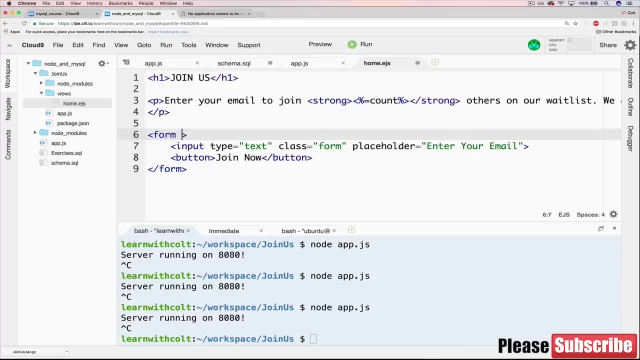 So there's no suspense here. We create a form element And the first thing we can do is add in method, and method We will set to be post could be all caps, all lowercase, doesn't matter, You'll see both. And that is saying that when this form is submitted from this button. 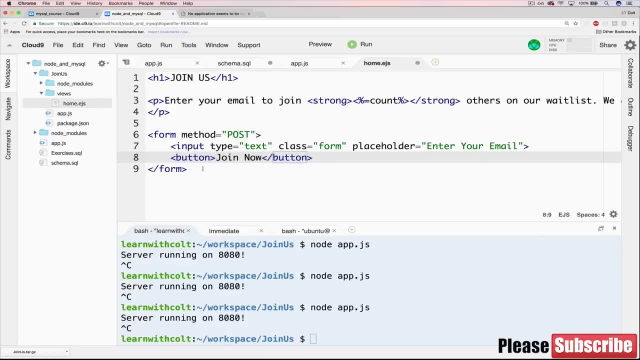 the last button, or if a button is the last thing in a form, it will automatically submit the form. So when it's submitted it's going to be a post request and we'll send it to a route that doesn't exist yet. So we send that with action equals, and then we could send it slash. 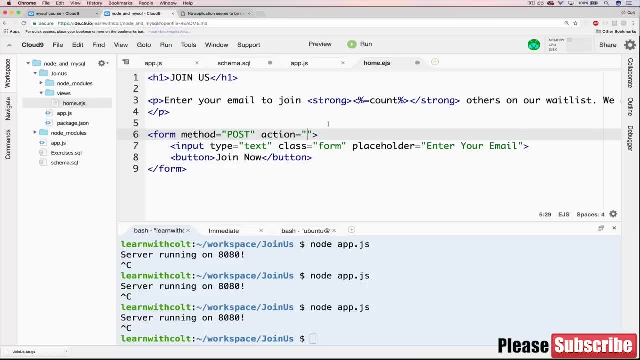 But that would just redirect us back here, except that needs to be a get request, so we'll get to that in a moment, But we could do slash register will make up a route that doesn't exist, So right now this form is going to take us to a page that doesn't exist. 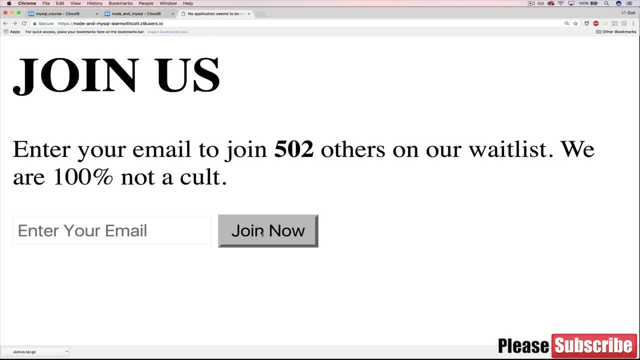 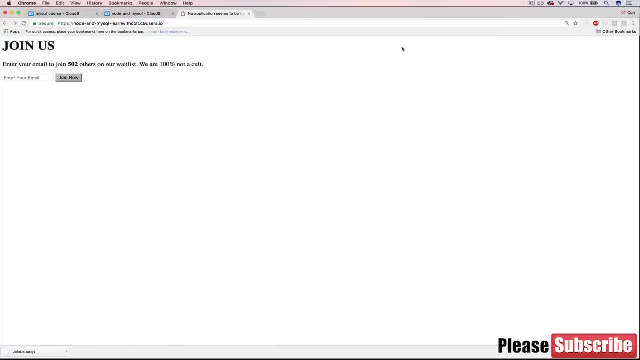 And if I try it Massive, Oh, this is still much bigger than it is in reality. it's about this size, but that's harder to read, so I'm just increasing the font. So if I enter something in here, click join now tells me cannot post to register. 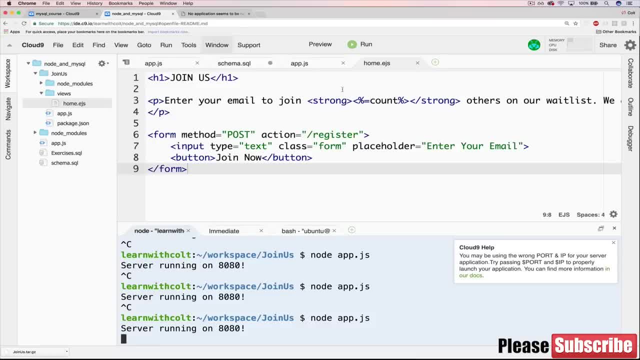 Great. So we need to define a post route to register. And again, the reason we're doing post is it allows us to send the form data. But what I could also do if I did a get request, I'll show you what happens. We already have a get route defined, a couple of them. 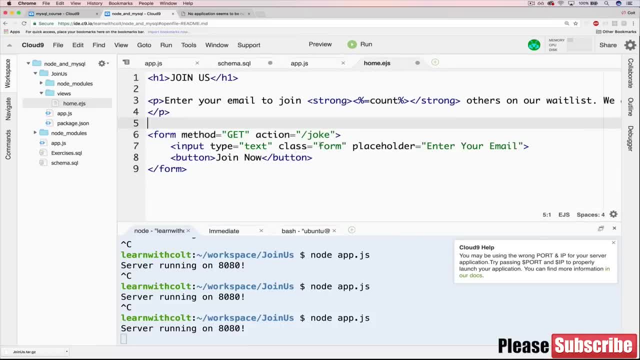 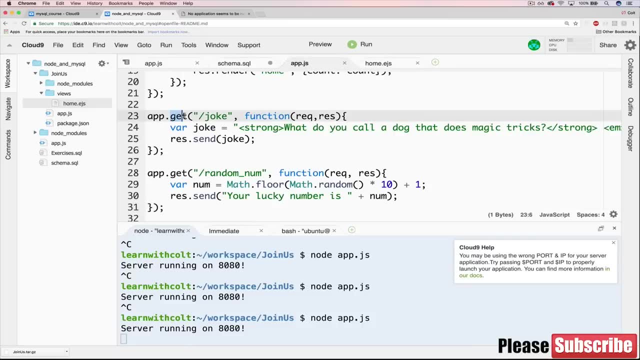 Let's do a get request to slash joke. So what that means is that when this form is submitted, it's going to send the data to slash joke as a get, which we already have. That's what this get comes from: app dot get slash joke. 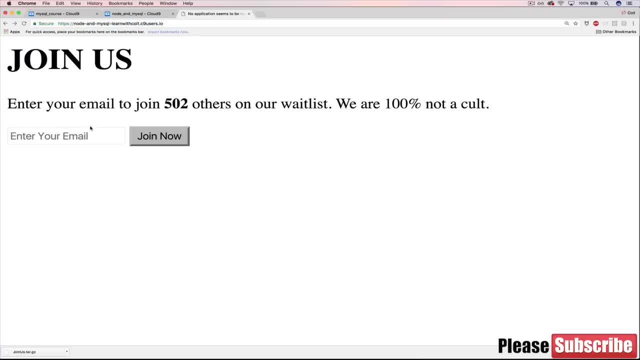 So if I restart and try it again this time, if I enter whatever there and I click join now you'll see it takes me to slash joke. There's also a question mark here, So that's something to consider. What's happening is that our data isn't. 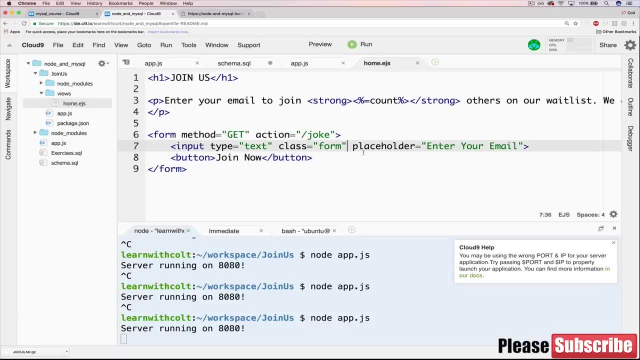 being sent because we're not giving it a name to be sent under. So what we do is assign our input here a name, and this will be the label for whatever. this is right here, which is email, So that's the best thing we could put there: Email. 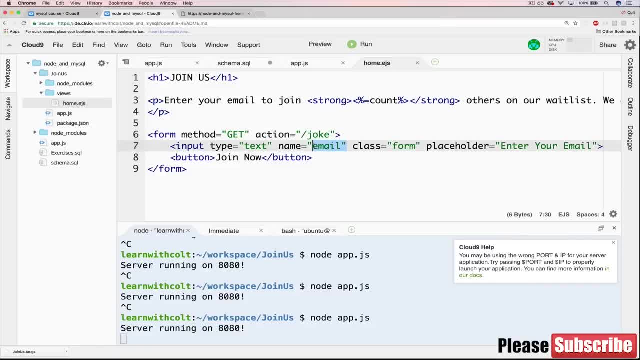 So when our data is sent off by the form, it will be referred to as email And there's only one piece of data that we need. If we had multiple things in our form, we might have email and first name and last name, and they could all have a name. 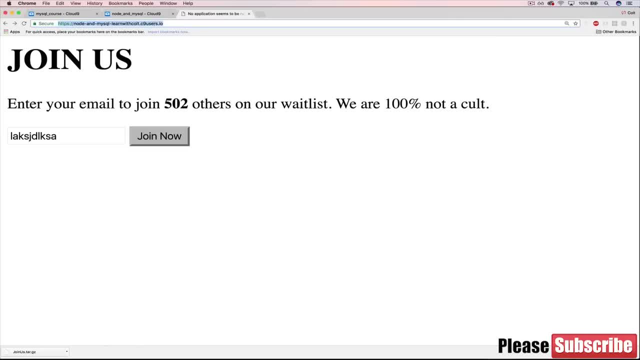 So now if we do it actually don't need to restart the server to do that. But now if I do blah at Gmail dot com and I hit join now notice that my URL. it's hard to read but it says slash joke. 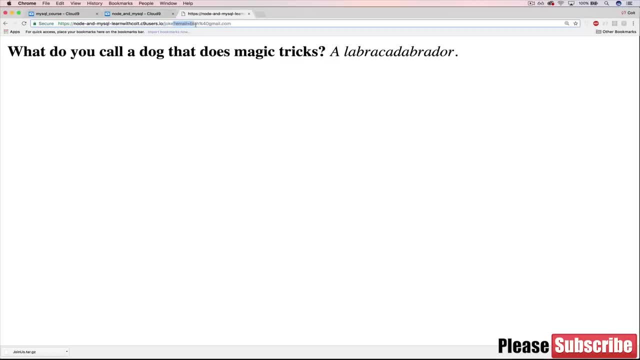 We sent a get request to slash joke and then it appends: email equals blah percent Forty is what it's doing for the hat sign Gmail dot com. So you can see our form data is making it here to a different request, But this is not a post request and we want it to be a post request for. Really, the main reason is that we don't want our data just to be appended like this in the URL. We could get away with that. The standard way of sending data from a form, if you're adding it into a database, is to do it as a post request. 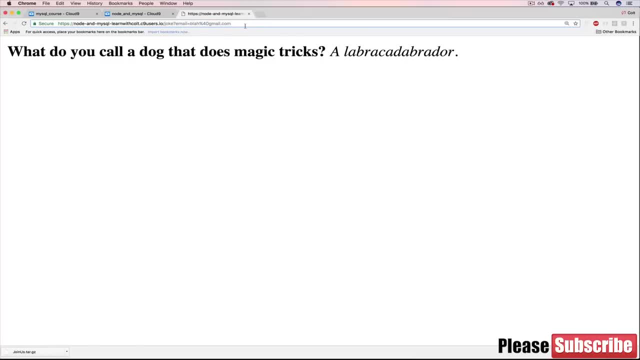 This is known as a query string. There's a lot of terminology here. This doesn't matter. We don't want it to work this way. I'm just telling you that it's not a conventional, It's not a good practice. If you're doing like a search form or something, this makes sense. 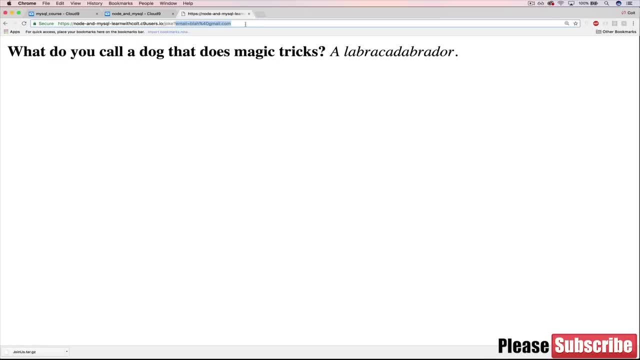 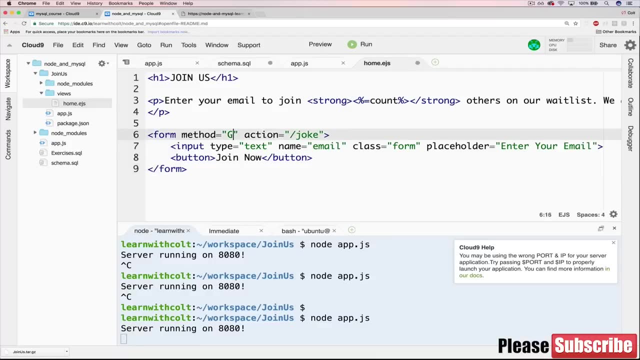 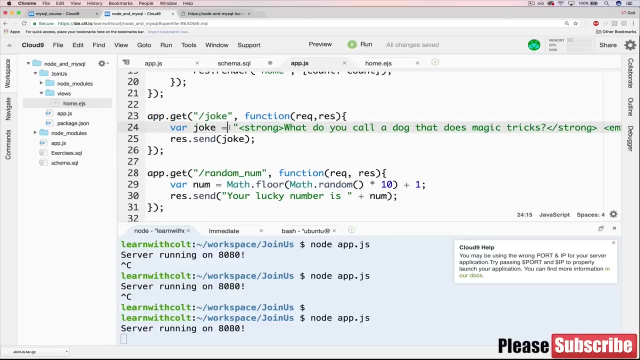 And you may have noticed, search forms and search results will often have query strings after the route. We don't want that. We want to send our data using a post request and not to slash joke, but to slash register. Now the problem is: how do we create a route that will listen for that? 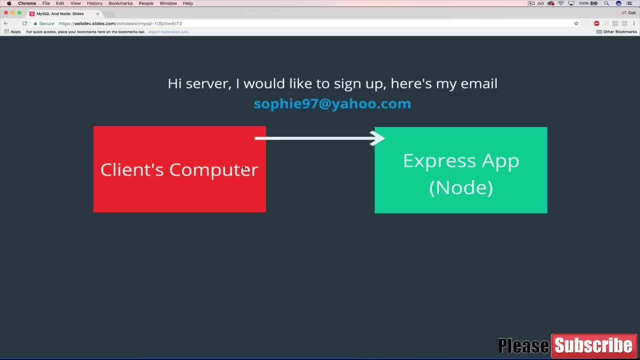 Essentially, what we're trying to do back to this handy dandy animation- is something like this: Hello Server, I would like to sign up. Here's my email. past the email to the server And then our node app or express app is: 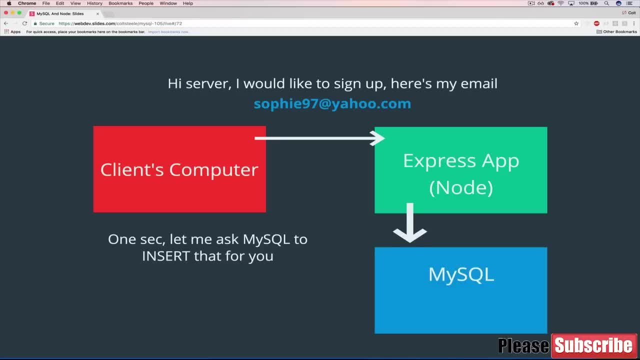 going to take that email and run an insert query with my SQL. My SQL, hopefully, says: great, it worked. Then we get back either something like this: Thanks for registering page, or we just redirect back to the home. So we'll decide on that. 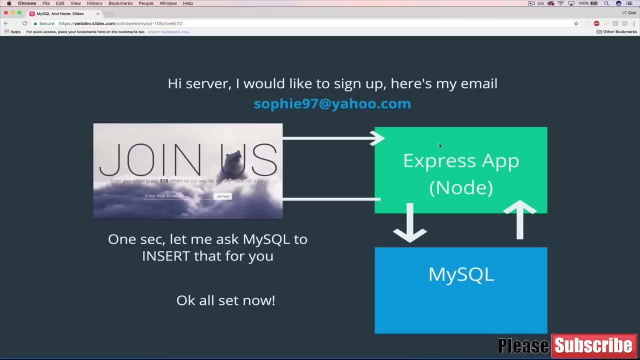 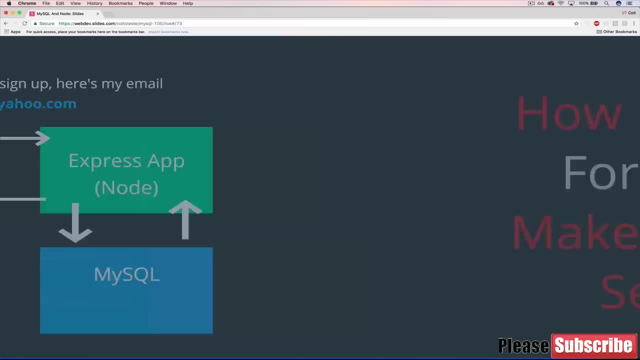 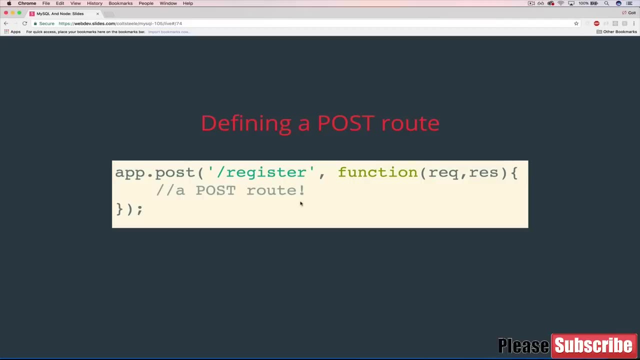 So how do we get it to, how do we get the express app- the right side here in the green- to accept this email or to even know if it's being made to slash register With this app dot post? this is how we define a post route. 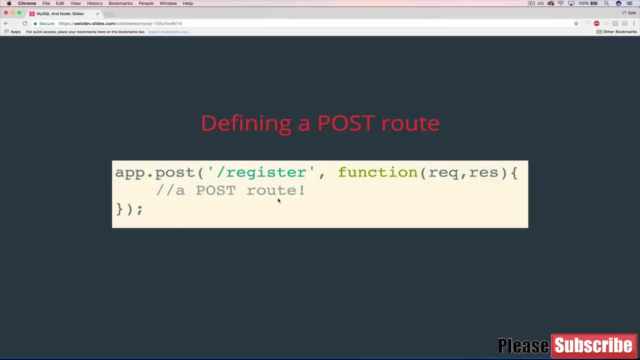 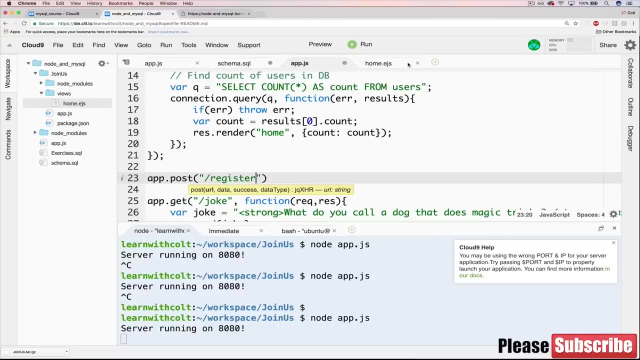 just like a get route, except it's app dot post. Everything else is the same, So let's do that now: App dot post slash register, which needs to match whatever we put here. So if this was registration or create user, Then this needs to be registration or create user. 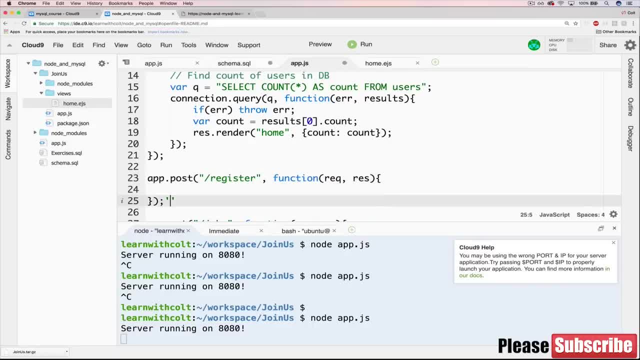 And our same request and response. This will only be triggered when a post request is sent to slash register. So just to prove that, let's do a console dot log post request sent to slash register, just like this. And now, if I restart my server, 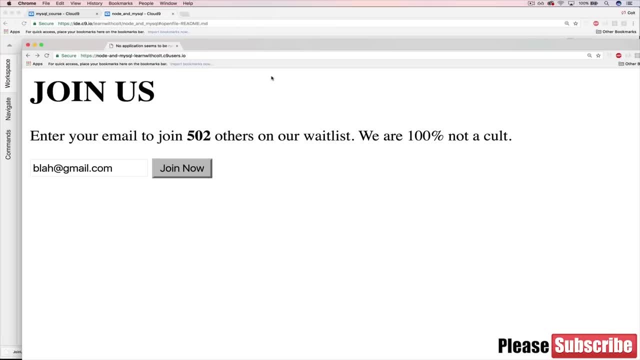 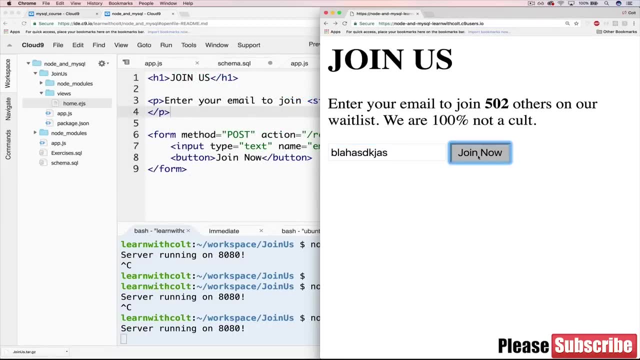 If you go back here, if I submit this form, I'll make it take up half the window here. So if I go down here and I go here and I type whatever I want in here and I click join, now notice that we get our post request sent to slash register. 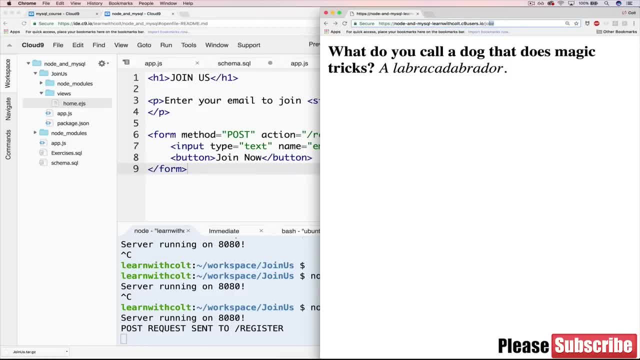 And if I try and get there another way, like by just going to slash register, this is sending a get request. We haven't actually discussed that, But when you just go click on a link or you enter a URL manually, that is sending a get request and that's why it's telling me it cannot get slash register. 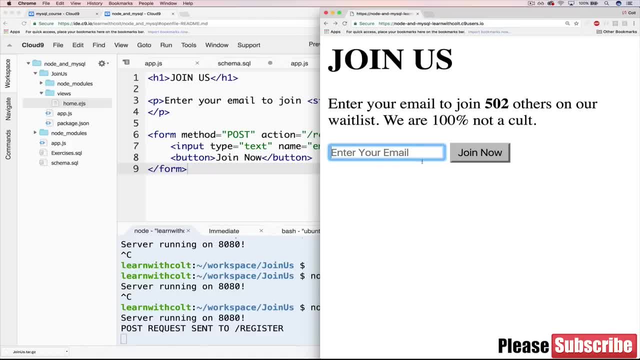 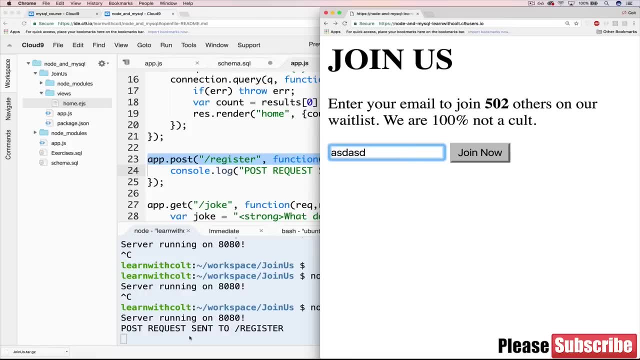 So essentially, the only way that we're going to be able to- in this case, that we'll be able to get to this route here and trigger this code is through the form. So one more time, put something in here, Watch down there. 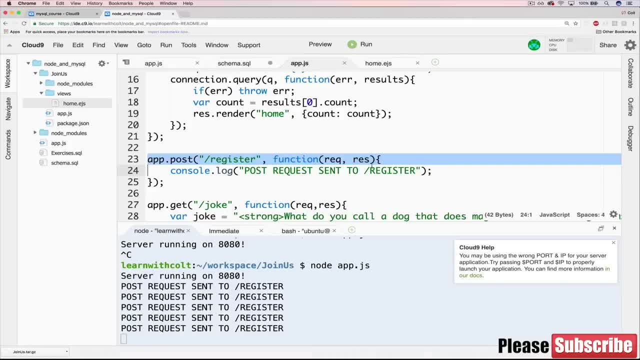 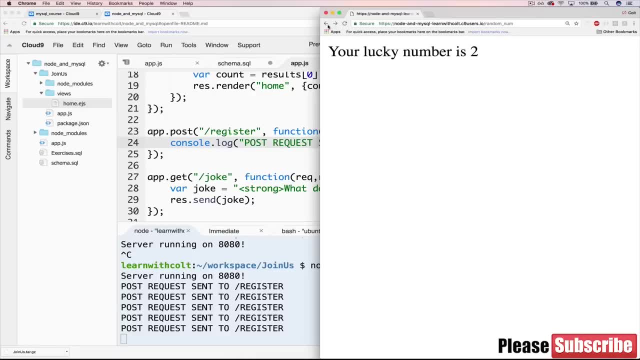 A post request is being sent every time. So what we want to do now is be able to extract the data that's being sent, And for now, you have to trust that it's being sent, that our form data is being sent. We don't have a way of seeing it. 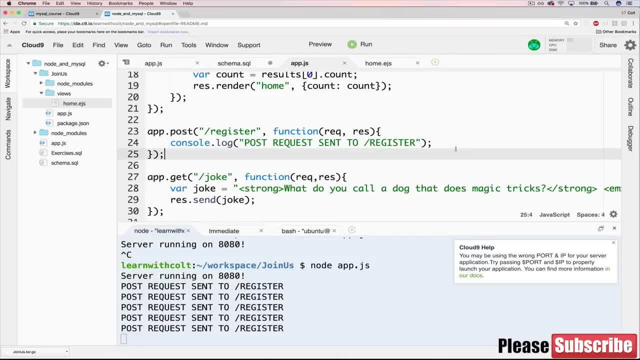 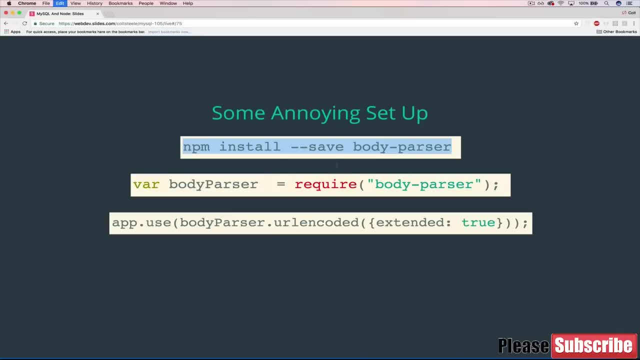 And the way that we see it. oh boy, it's a little bit complicated. I'm going to walk you through the steps here. This is the annoying setup we have to do. So we have to install something called body parser, And I won't waste much time talking about it. 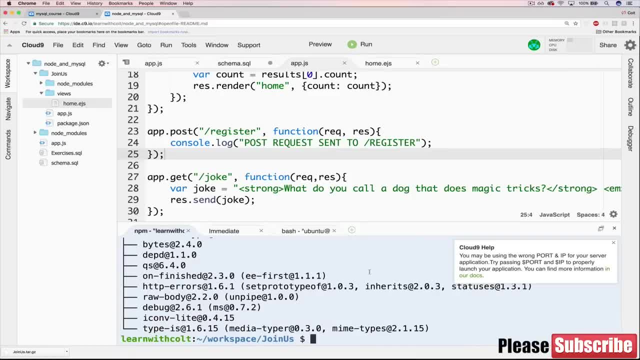 What's happening is that Express is a lightweight framework, which means that it doesn't come with everything that you would possibly want pre-installed. So we have to go and select certain things, And body parser is one. What it does is it parses the request body. 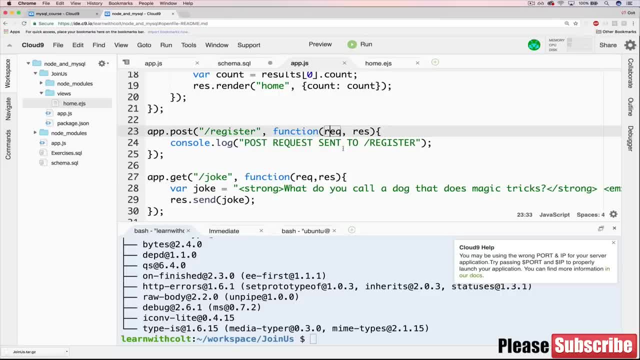 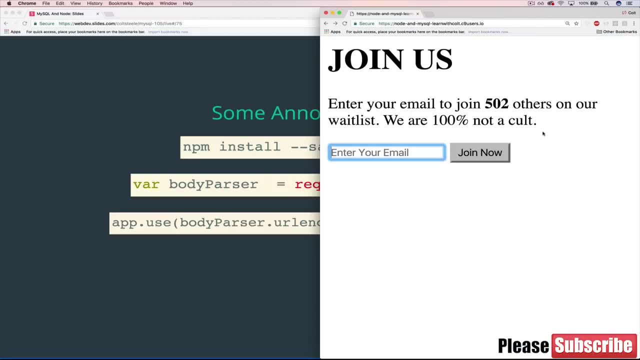 So remember that when a request is sent, there's all this. it's just a giant block of text and somewhere in there it says: email is equal to whatever we typed in here. But it's in a giant block of text, It's not. it's not JavaScript or anything. 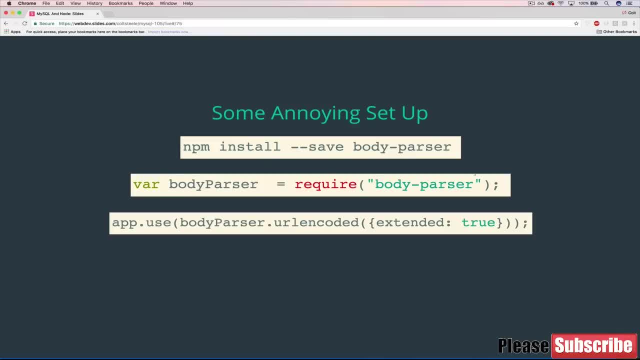 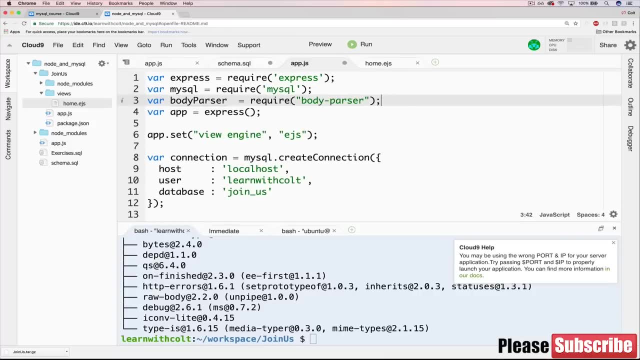 So body parser will intercept that and turn it into JavaScript that we can then use and manipulate. So then, what we need to do- and I'm just doing this quickly- it's just copy and pasting: importing body parser. equals require body parser. 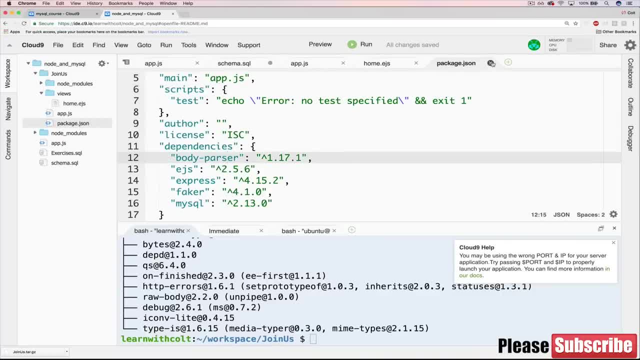 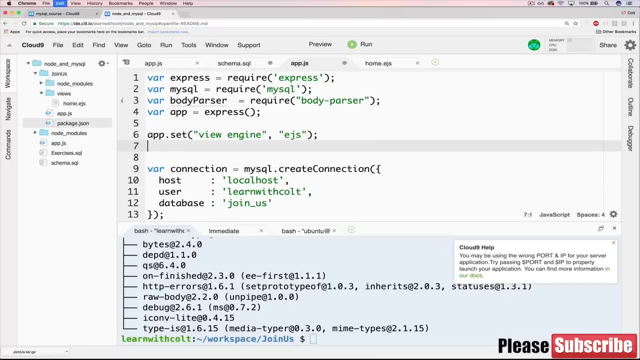 So we can save that. make sure our packagejson has body parser in it. Then, finally, we need to tell our app to use it. So I'm also just going to copy that line and put it next to appset. so we have our configuration lines together. 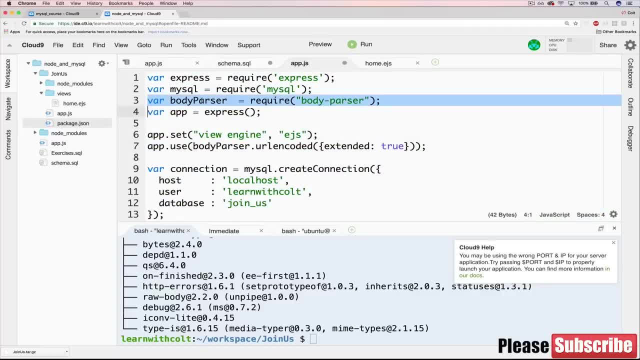 We're not going to go into detail on this line, but this is just requiring body parser doesn't do anything. we have to tell Express- which is app- right, App is from Express- that we're using body parser And this now allows us to extract information from post requests. 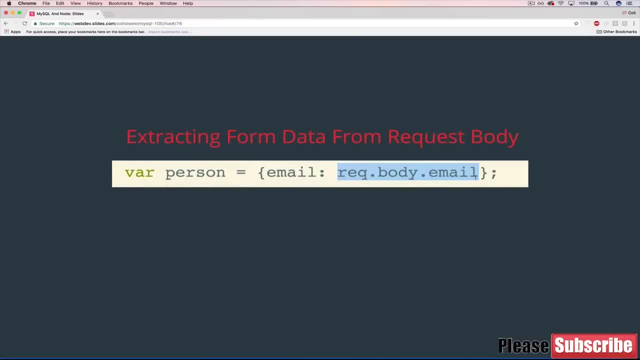 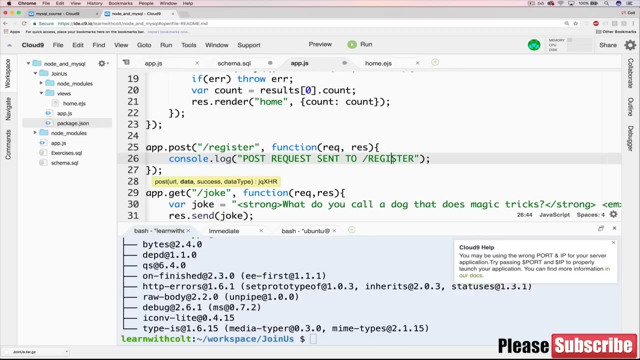 And here's the magic line: Requestbodyemail. So what this will now store in the request body in that post route under email will be the email address coming from the form. So let me show you that If we go to our post route for register rather than consolelog, post request sent. 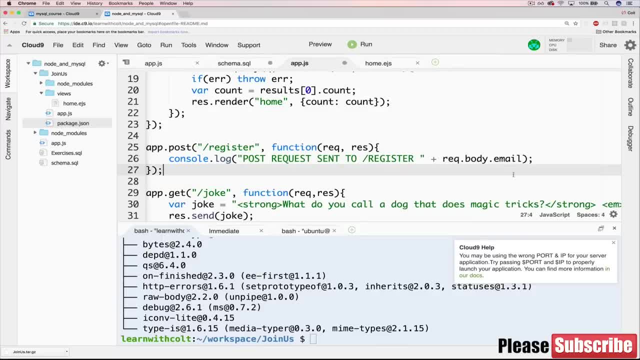 to slash user. we'll also add plus requestbodyemail Email is how about that, Requestbodyemail? Okay, So we definitely need to make sure that we have name equals email, and then we should be good to go, assuming our install went okay. 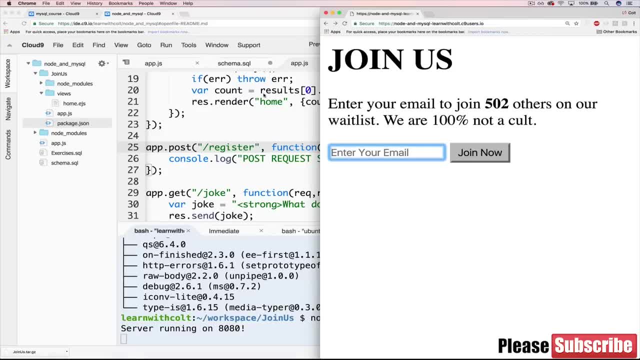 Let's start the server again. It looks good. Let's go over here. I'm just going to refresh this page Now. I'll type c at gmailcom. Join now. And what do you know? Post request sent to slash register email is c at gmailcom. 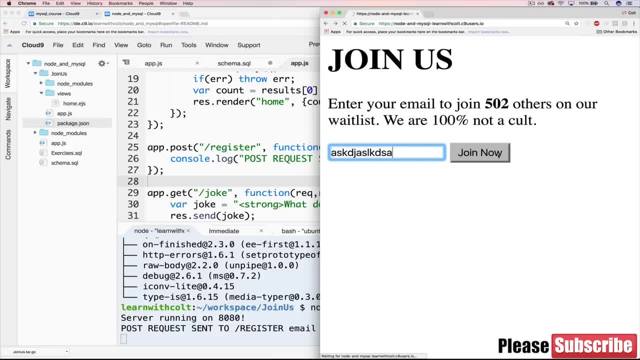 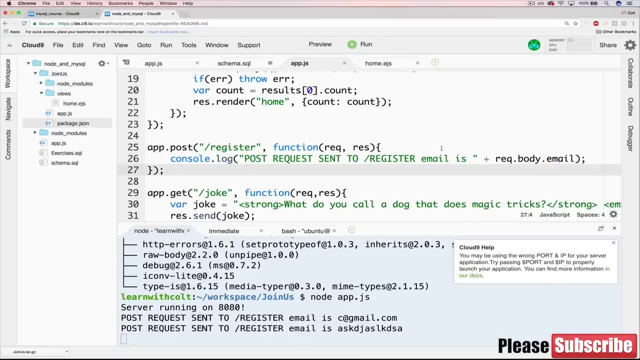 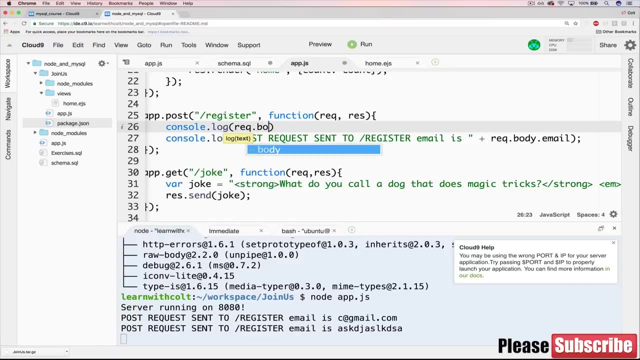 So whatever is typed into that form is being stored in requestbody as email. So body parser is doing the heavy lifting for us here. We had to do kind of a couple of annoying lines, but let me show you what body looks like. So requestbody on its own. 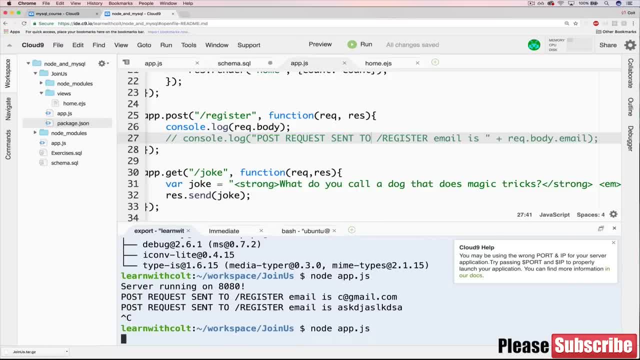 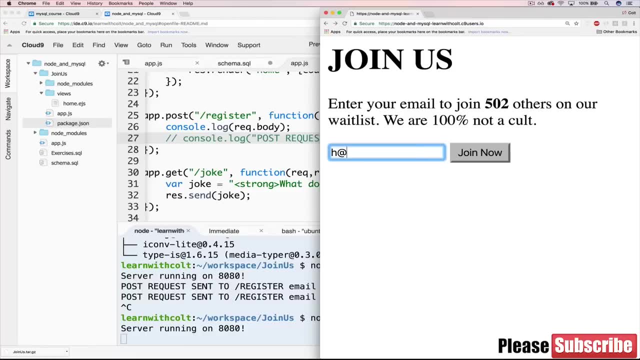 So I'm going to comment that line out. We're not consolelogging anything. Now, if we go back to the form refresh and I type I don't know h at gmailcom And I click join now, This is what our requestbody looks like. 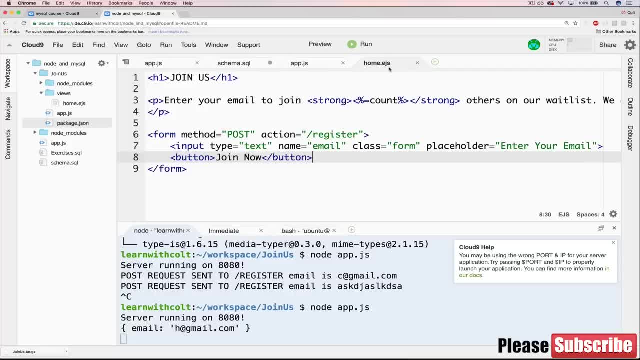 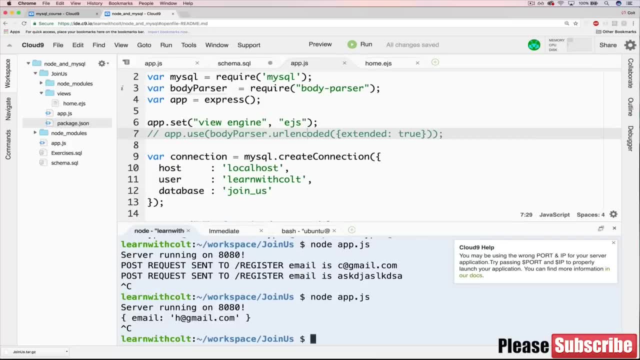 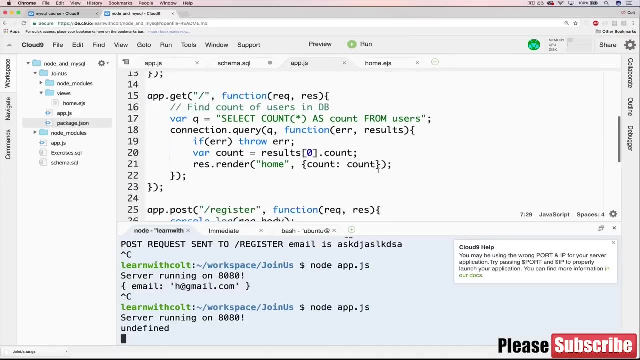 Email is: h at gmailcom. Again, email is coming from here, But if I get rid of body parser, let me show you what life is like without it. And I do the same exact thing. h at gmailcom. Now there is no requestbody. 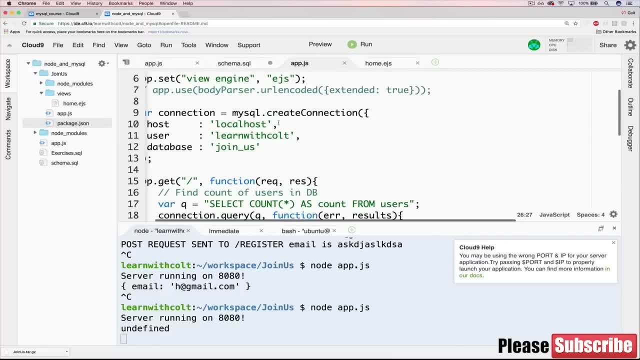 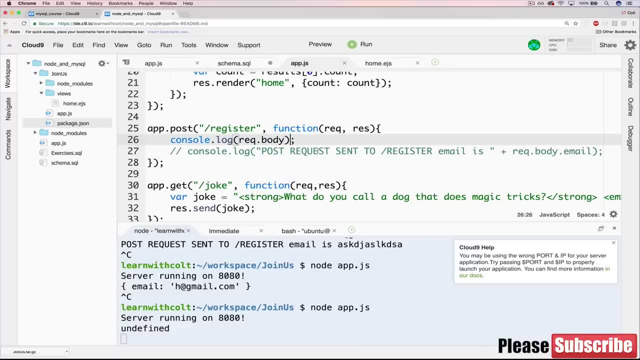 It's undefined. I did everything else the same. So just this single line telling our app to use body parser is what allows us to access requestbody. So the information is still being sent to Express, but Express is just not doing anything with it. Requestbody is what we need. 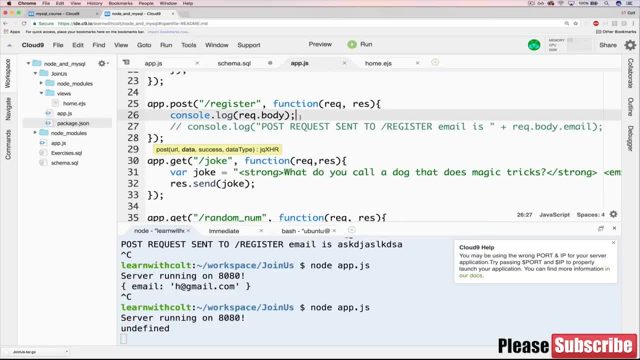 along with this body parser line to start using it. So it's kind of confusing, but that's the whole. ethos of Express is that you add the tools you need as you need them. So rather than giving you everything at once and you might only use one out of 20, 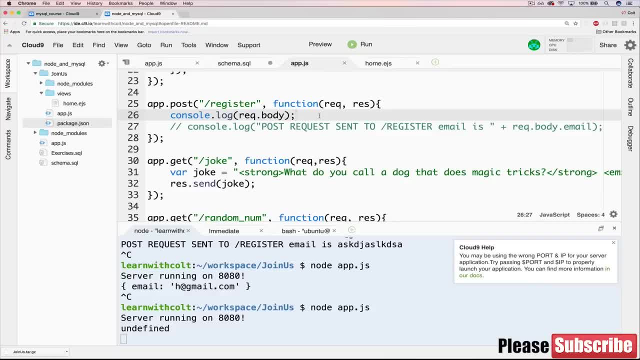 things. it gives you one thing, two, three things, and then you go and grab the other things you need. So if you need post request, you need a requestbody to be filled in with data, Then we need body parser. OK, so then, all we really need to do now 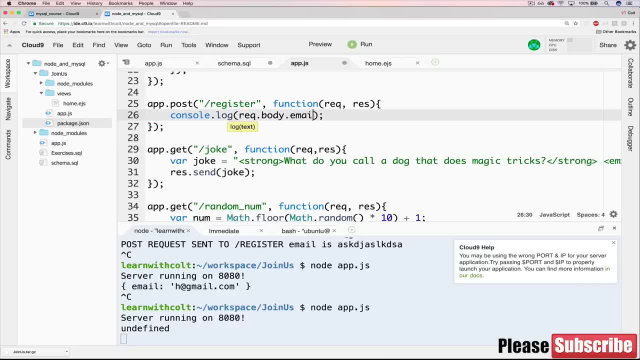 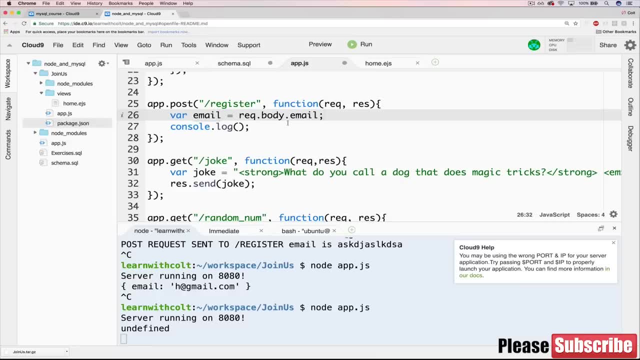 if we're isolating requestbodyemail, that's the email that's being sent. Let's save it to a variable. Now we just need to insert that: make a new user, which we've already seen how to do, and I won't make us type it from scratch, but hint, hint. 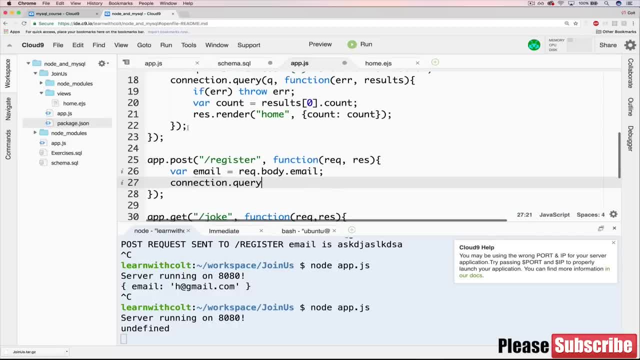 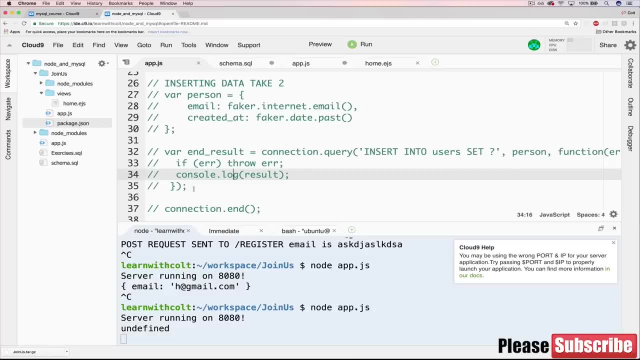 we're going to be doing connectionquery And we've already seen how to do the query. It's going to be an insert into. if we go back, let's just copy this code here. This is what we've done in the past, where we inserted a single user. 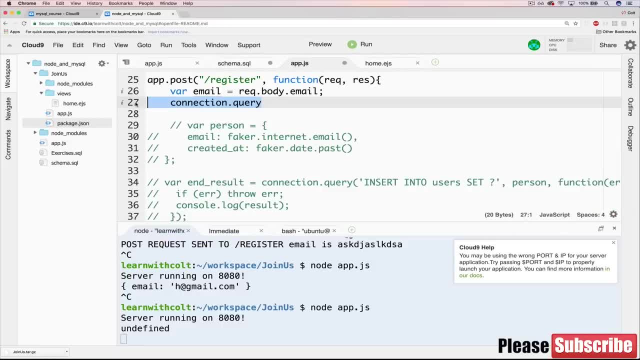 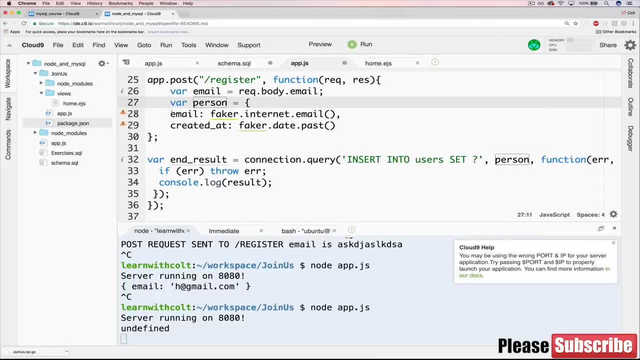 Go to appjs. So I have it commented out. I'll uncomment it. There's a couple of things we're doing. The first: I made a variable called person with an email and created that. But we don't need that created at anymore because this is for faker. 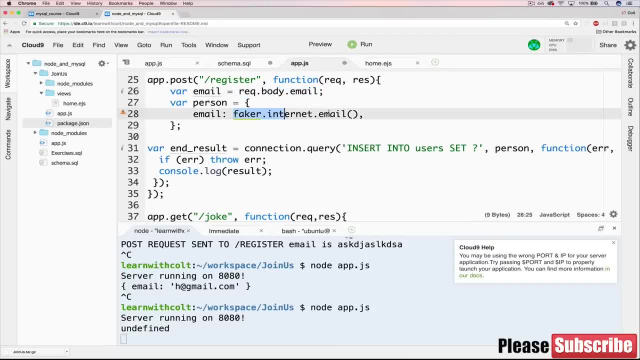 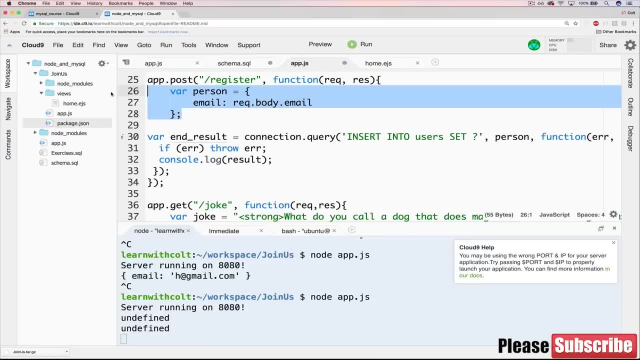 We actually have a real created at, And then for requestbodyemail, we can just replace that. OK, so we can get rid of that variable too. So this is just preparing the data to be inserted. We'll have a person object that has an email: requestbodyemail. 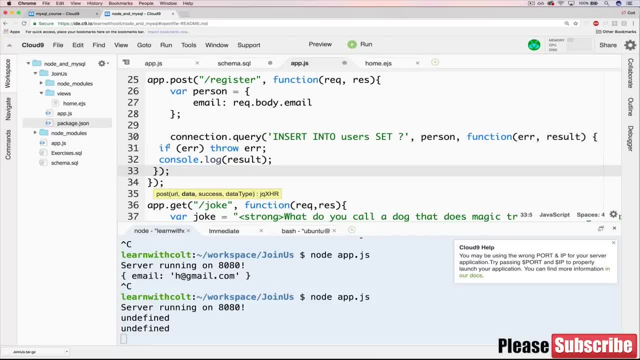 And then all we need to do here- we don't need to store it in a variable- is just connectionquery insert into users set, we pass in person and then we have our callback function. So this is review. We've already seen how to insert. 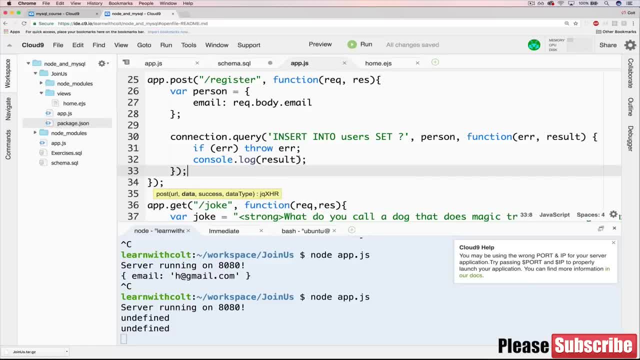 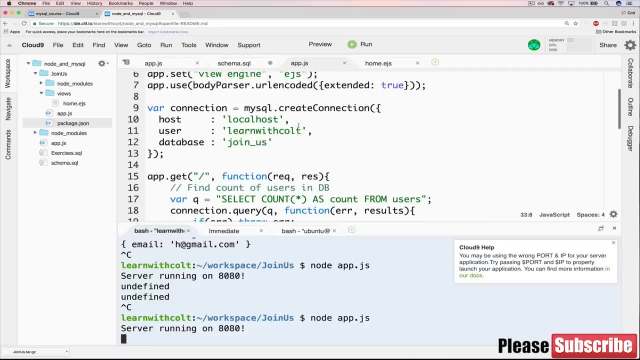 So I want to spend a ton of time on it And, rather well, we can start by just consolelogging the result, which will be a lot of stuff, hopefully. Let's see what happens. now. We have body parser working again. 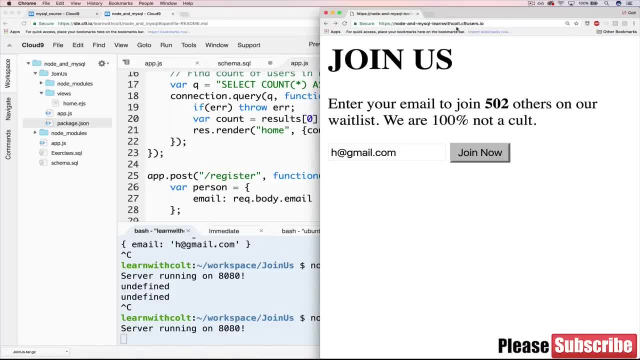 OK, good, Now if I go over here this time, it will insert a real user. So let's do a more serious email address. Well, I guess that doesn't matter. How about Miranda? Let's not do all caps. 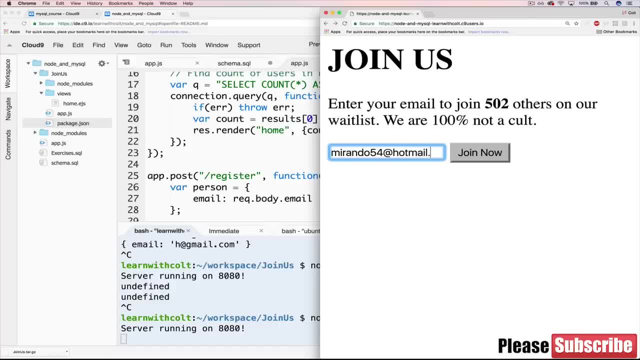 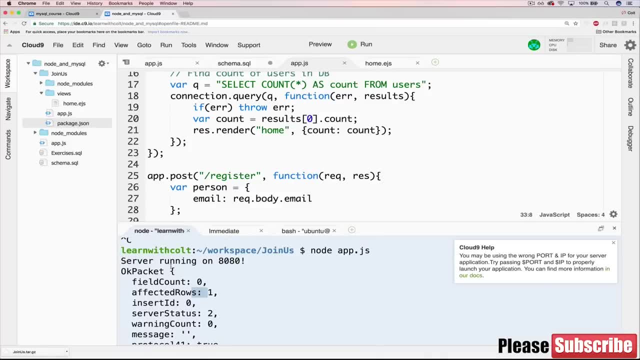 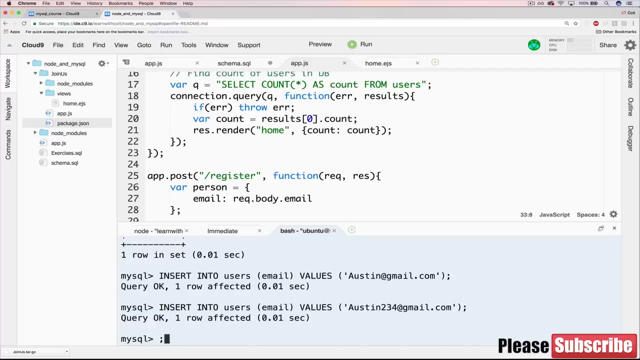 Miranda54 at hotmailcom. Miranda, There we go, Join now And look what we get back: Affected rows one, It's this: OK packet, all this other stuff. And if we went into our MySQL, if we wanted to do a select star. 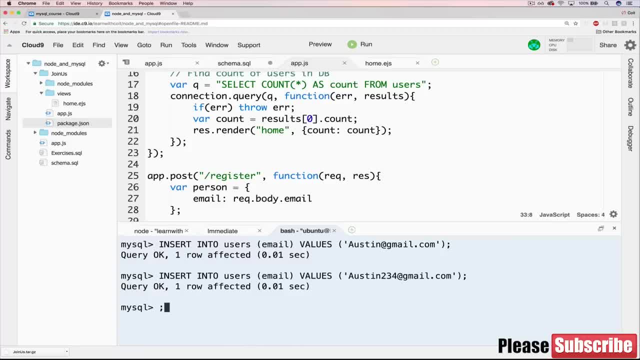 well, it's going to take a bit, Let's do. let's have to type it ourselves. select star from users. Order by created at limit one. We don't have a user's table and all caps. Oh boy, we get the wrong user. scared me for a moment. 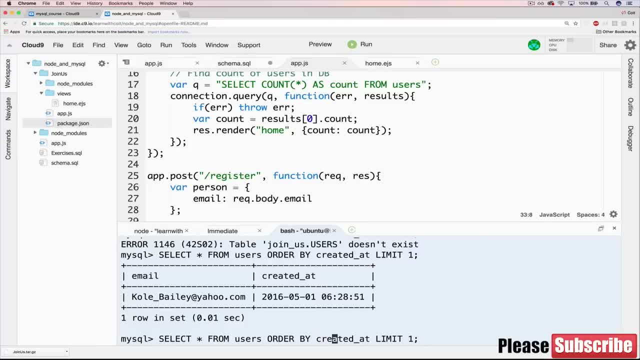 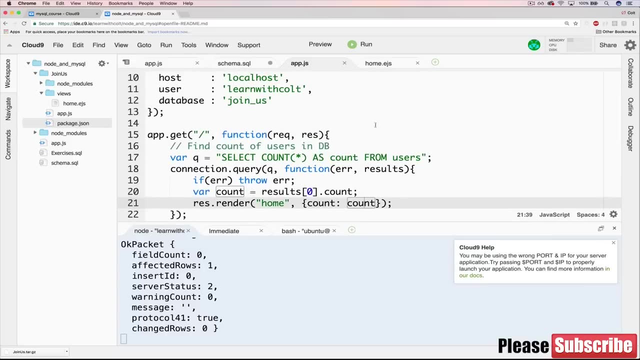 We need to also change the order at, or order by created at, to be descending. And here we go, Miranda54 at Hotmail. So it worked. Long story short, it worked And we're pretty much done. The only other thing we have to decide is: OK, our web apps is just kind of hanging here. 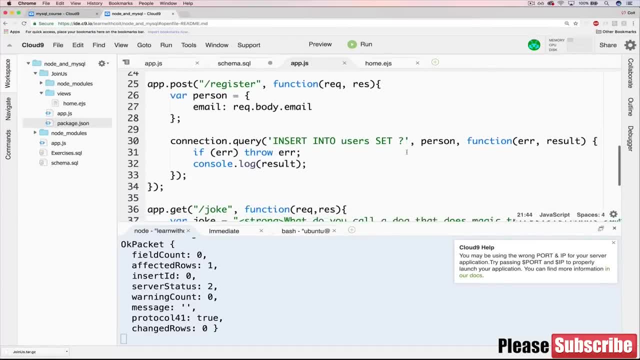 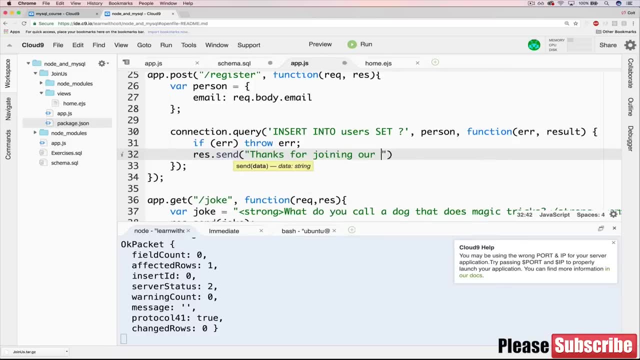 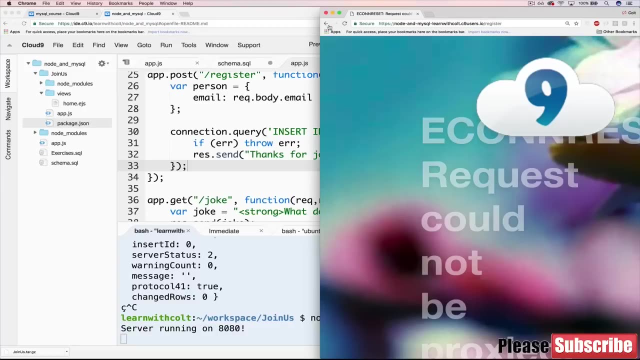 You can see that. What do we do next? We could either do something like a ressend Thanks for joining our waitlist- Let's say we can start with that, And if we restart the server, do it again. Have someone try and sign up the new email, let's say Jane Doe. 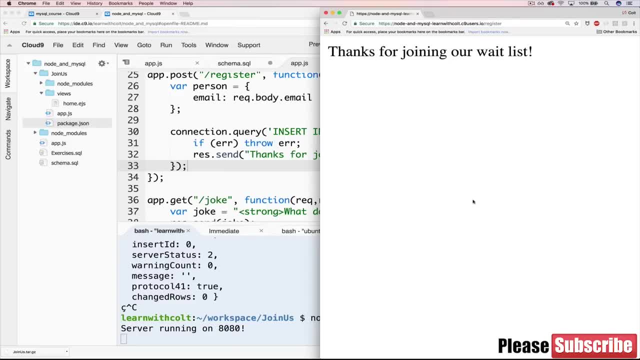 At gmailcom. Click Join now. Now we get thanks for joining our waitlist, So it's totally up to you how you want to structure this part. What I'm going to do is just have it redirect back to the same page, to the original page here, and we'll be able to see 503 or 504.. 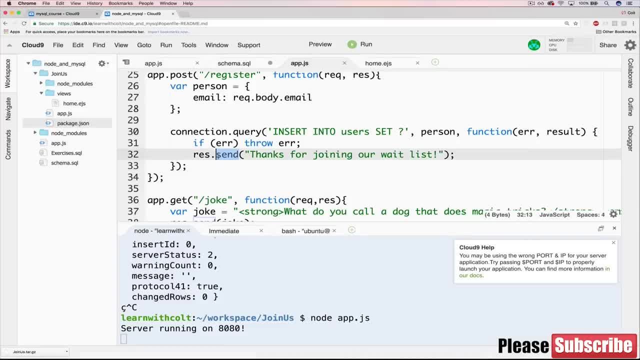 It's really up to you. This is how you. you wouldn't use ressend. You could do a resrender and you could make a thank you page if you wanted to, But what I'm going to do is show you another line, which is just resredirect. 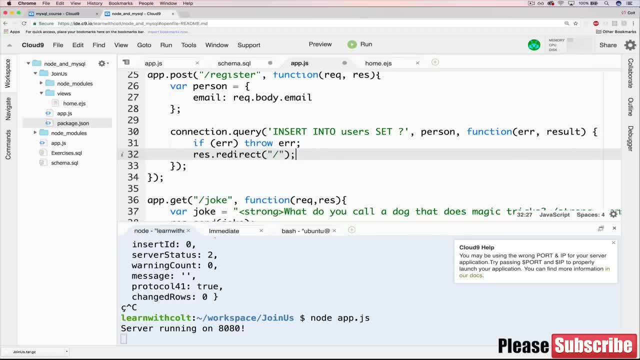 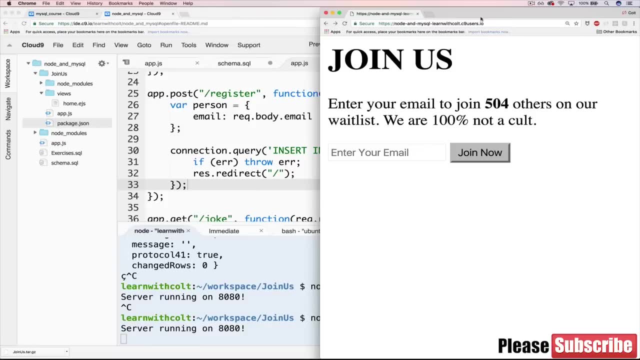 So res being response up here, resredirect to slash, And that will just take us back to the home page. So effectively, what's happening if I restart one more time is we're on the home page. 504 is how many we just got from the database. 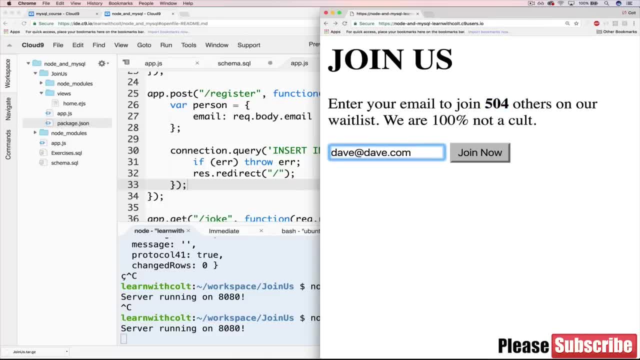 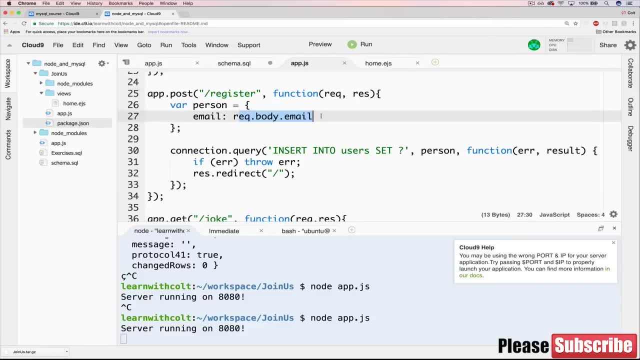 I entered a new one, dave. at davecom. I click Join. now It's going to hit this post route slash register. We're extracting the email From that form data in the body And then we're inserting it as a new person in our new user in our database. 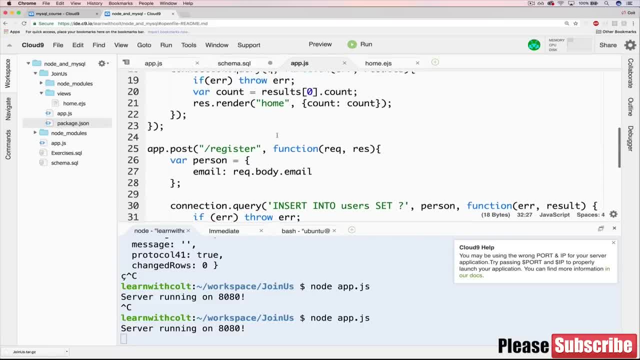 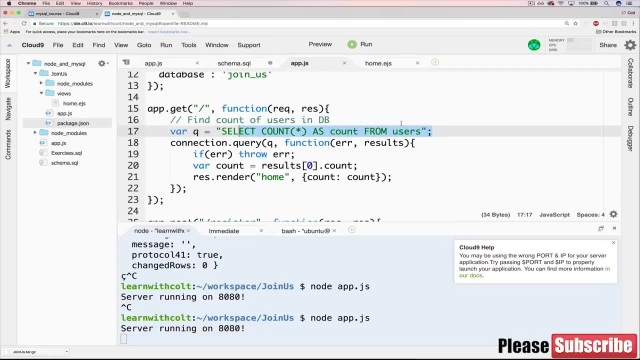 When that finishes, we're redirecting back to slash, which starts this whole process over. it's going to then select all the count of all users, then it's going to- oh, there's my cat. And it's going to render our home page with that count. 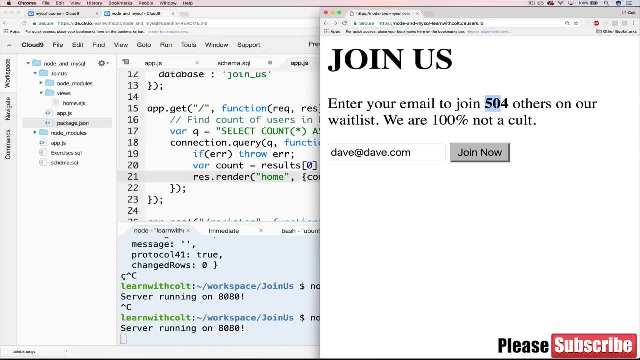 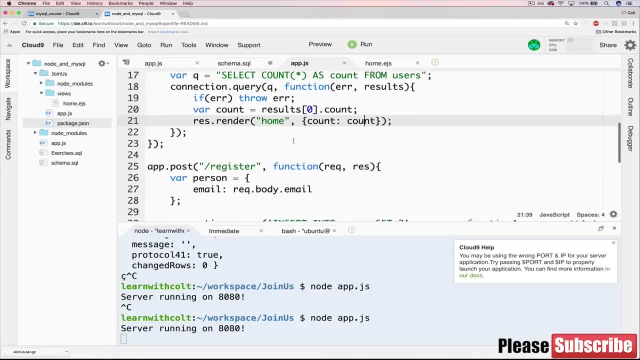 So to the user it will just look like this page refreshes And this goes from 504 to 505.. But behind the scenes a lot more is happening And there we go. OK, so that's awesome. Hopefully you think that's cool. 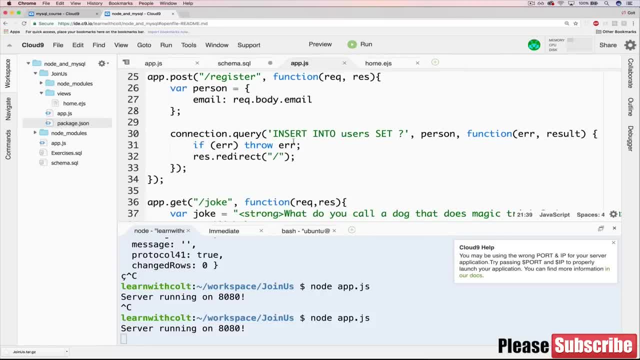 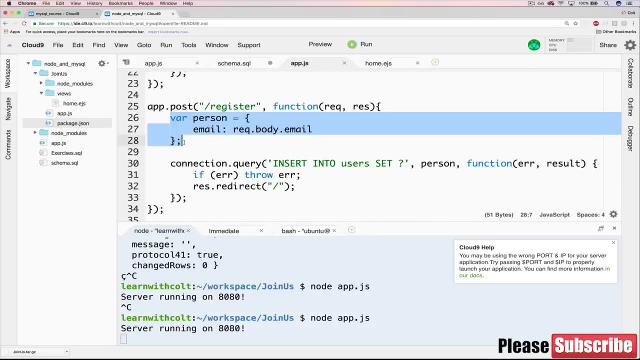 All we have left is to style it. If you would like a little bit more detail on the, the insert part- and I can go over that a bit more if you'd like- and what's happening here. But if you feel like you've got a grasp on it, you want to move on to styling. 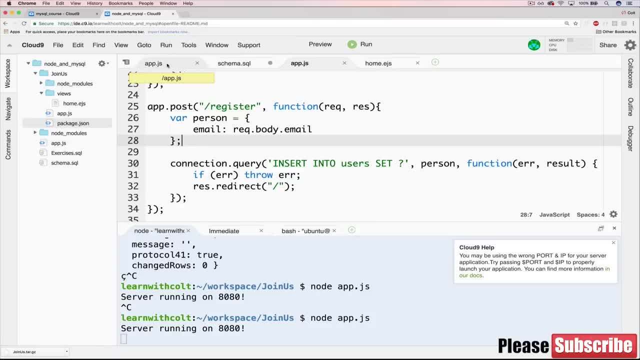 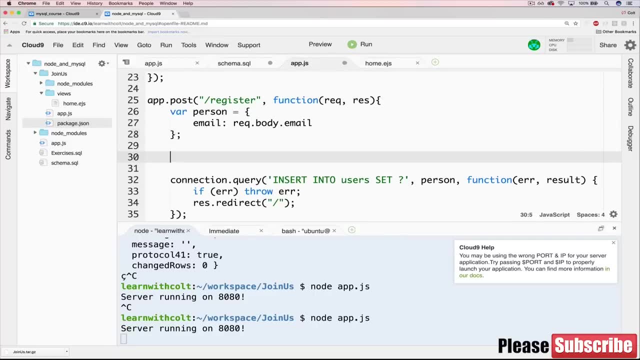 Go ahead. OK. So just to reiterate, we could have also done it a little bit more manually if we wanted to. We could have written a query like this: if I did VAR query and I could have done insert into users email. So this should be more familiar values. 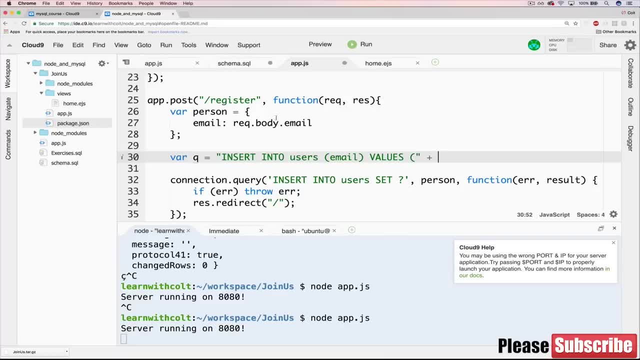 And then I would do parentheses plus Request that body email Plus clothing closing parentheses like that and that could be our query. So this would turn into: But let's say, request that body email is Dave at Dave dot com. It would turn into: 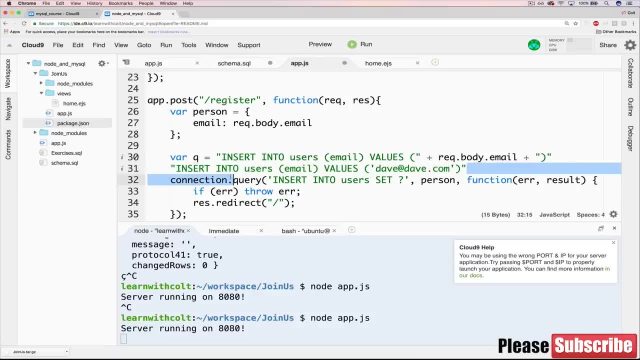 Dave at Dave dot com like that. So we could- we could also do this query this way and then all we would need to do is pass Q right here, if that makes sense. So that's another way of doing it, But this is kind of the standard way of doing it with the MySQL library. 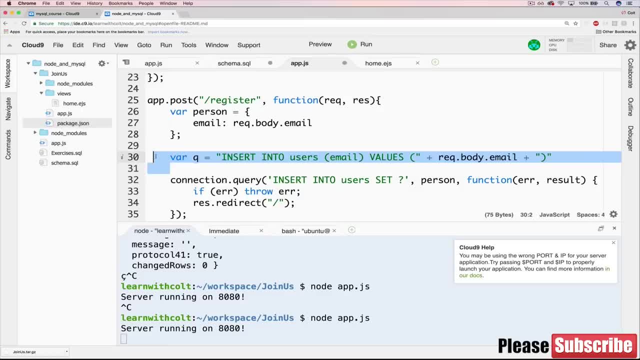 the MySQL package that we've been using, So I'm going to get rid of that. But either way, maybe the syntax is more unfamiliar if you don't know JavaScript, But this is what we already saw as to how to insert a single piece of information, a single row, into a table. 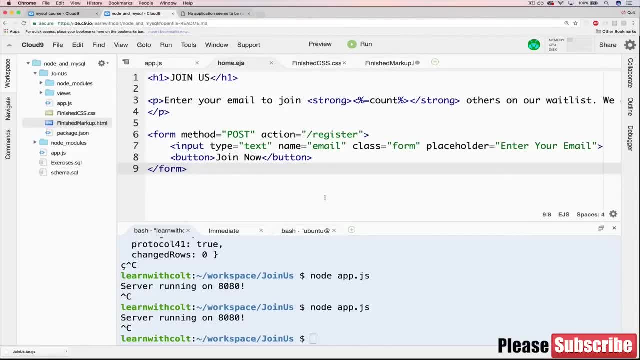 And it's working great. OK, so we're at the end of this project. All we have left is to style it, And it's kind of funny. I think for a lot of people this is the most exciting part, even though it has like the least. 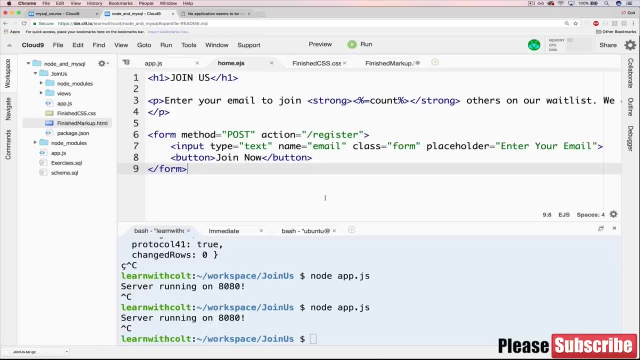 To do with the course, but I get it. It's nice to have something visual to make it look nice. If you know CSS, skip this. You can just copy the style sheet in. Take a look at what I did. This is not going to be, like I've said a couple of times, not a course on X. 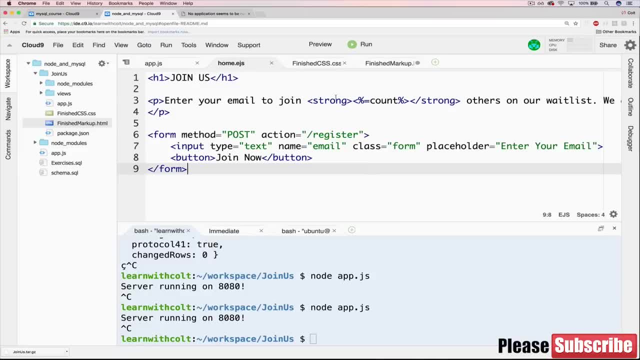 It's not a course on CSS, So what I'm going to do is, rather than spending two hours of video going over styling this one piece at a time and talking about my workflow and why I'm doing certain things, what I've done is just copied over the finish. 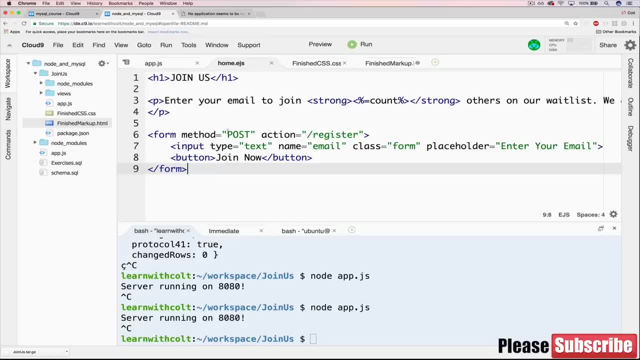 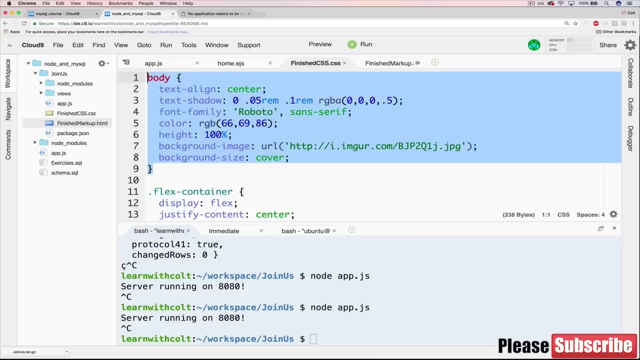 Style sheet and our finished markup. But we still have our empty market or basic markup and we don't have a style sheet. So what I'm going to do is just walk through and kind of copy bit by bit over and explain what chunks do, but not everything. 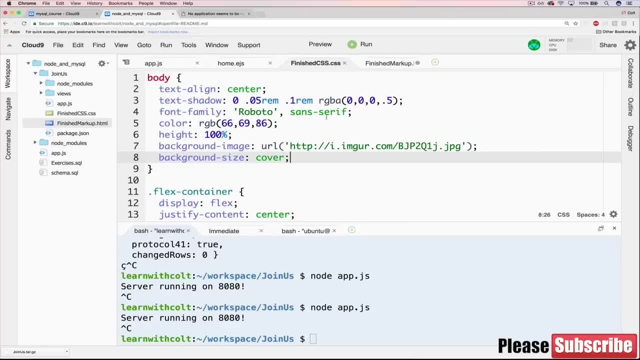 And these two files you can also. you can find yourself. They're not in, the slides are too large, but I've included them along with this video so that you can copy from there, unless you're someone who likes to type things manually, which some students do. 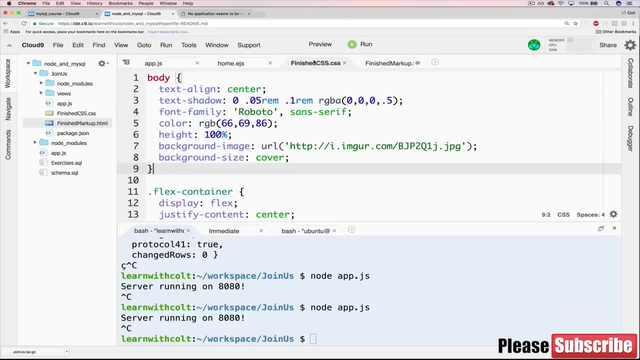 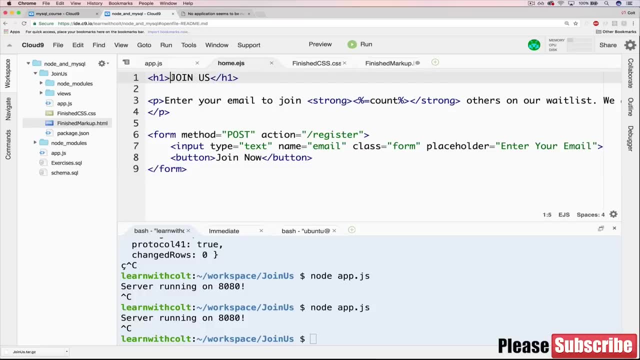 OK. So again, these are Two files that are not connected to our app. These are the solution files I'm going to refer back to, But for now we're stuck with this, our basic HTML, And we don't even have a way of styling it. 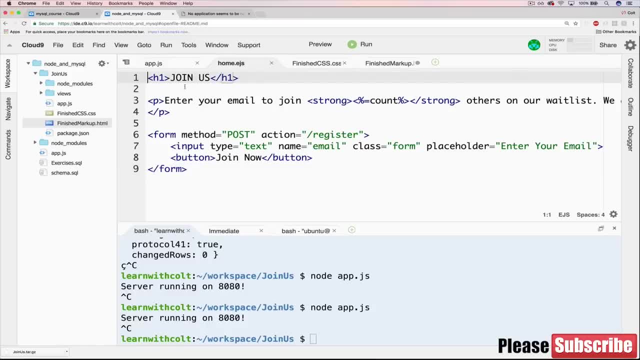 And for those of you who don't know CSS or know what it is, it's how we add style, color, font, images, how we add images generally, But it's how we can add a background image to something using CSS And the way we usually write, that is, by creating an external style sheet. 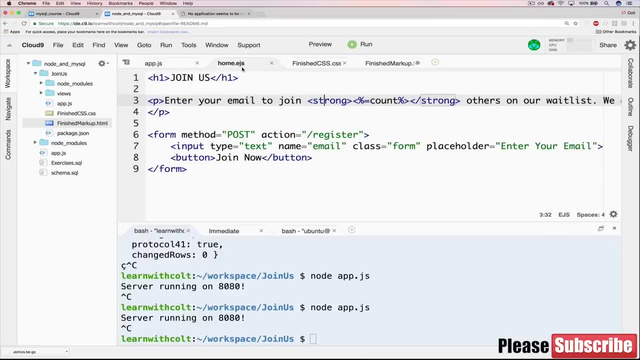 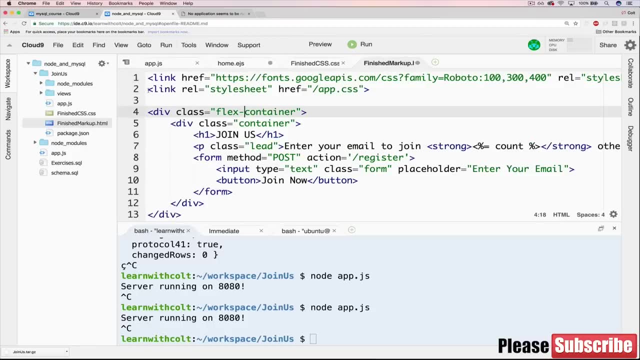 a CSS file and writing our styles in there like this. So we need a way to actually connect them And I'm not going to go into too much detail, But so usually what we do looks like this: We'd have a link. rel equals style sheet. 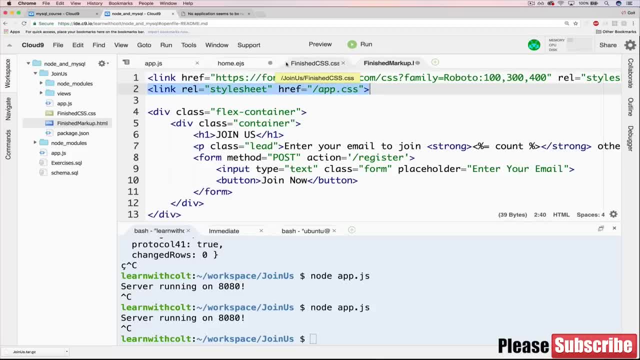 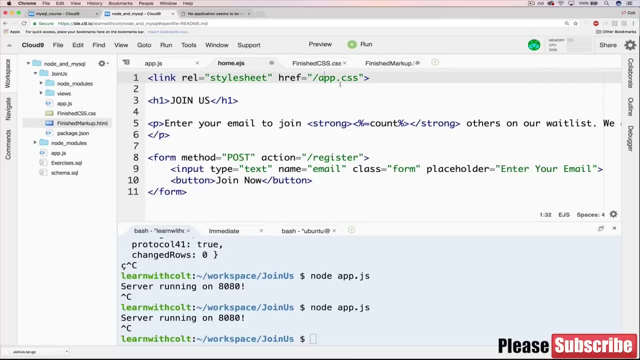 This is an HTML tag that includes an external style sheet. So if I do that and I just paste that in here, there's two problems. One: we don't even have an app that CSS created But to express isn't going to know about it. 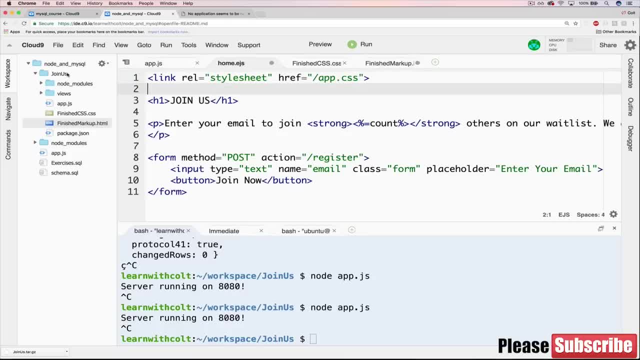 Hi Blue. What we can do is start off by creating a new directory, And this is just a conventional name. I'm going to call it public. That's kind of standard for a Web app, but you can call it whatever you want. 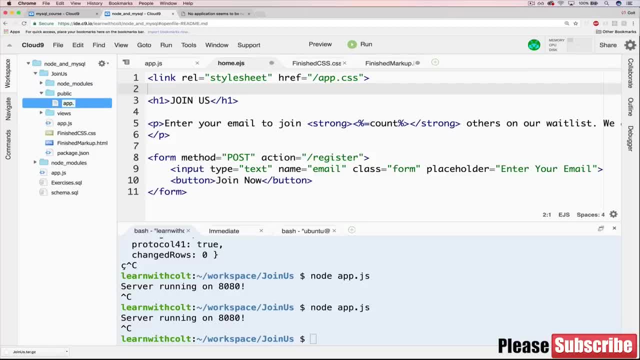 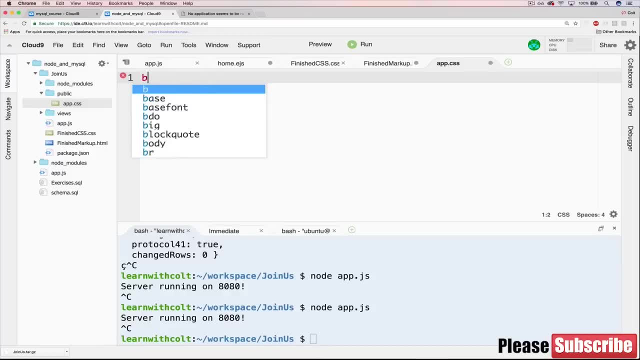 And inside of there I'm going to create a file called app dot CSS, like that, And then we'll put our code in here. And let's start with something really simple like turn the whole body, make its color purple, So all our text is purple. 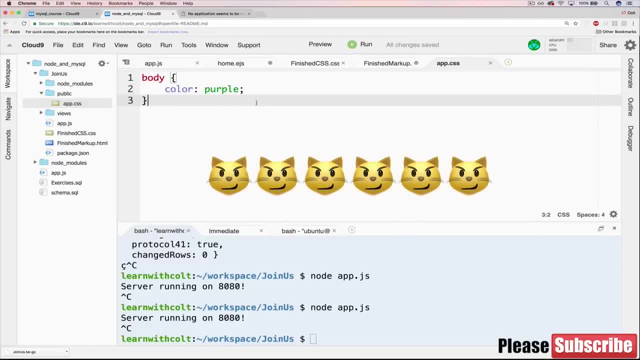 Like that color purple out, blue. Hey, my cat just attacked me. Hey, why don't you let me record? Okay, hang on, I'll be back. I got to handle this. All right, That's been handled. Crazy cats. 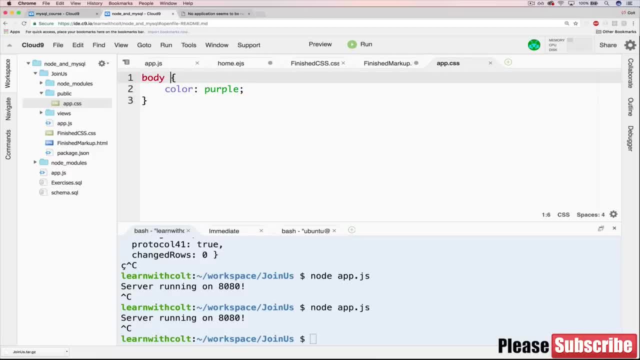 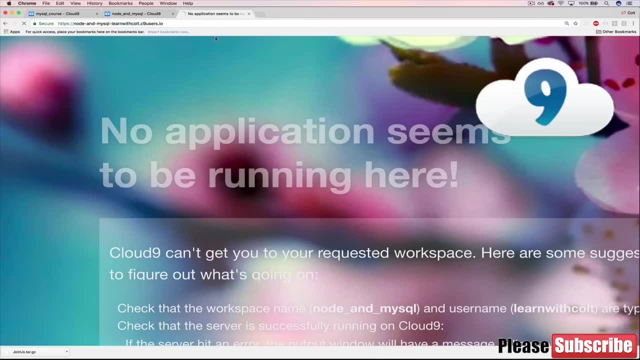 So, back where we were, we've got our app dot CSS body color purple. This is not connected to our app. If it were, then our text would be purple, but it's not. So how do we get it connected? Well, there's a problem. 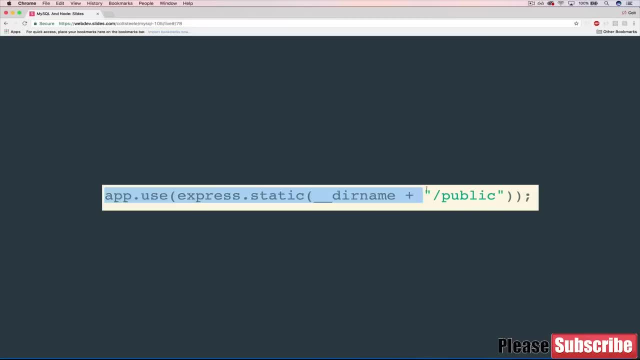 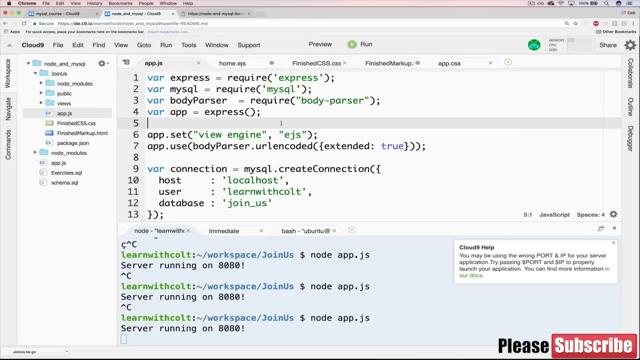 Long story short. we need to add this line. So this is another app dot use And this tells Express. If I go into our main file here, app JS, just add it with the other app dot use. keep all our configuration. 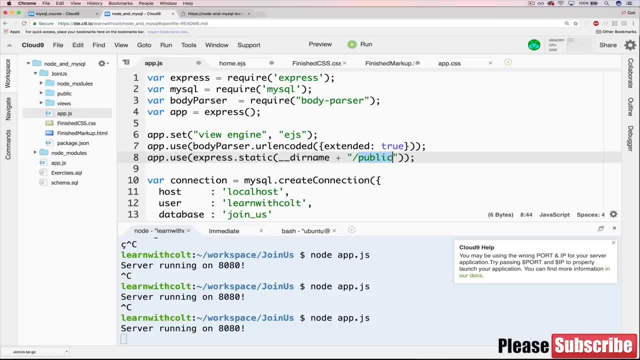 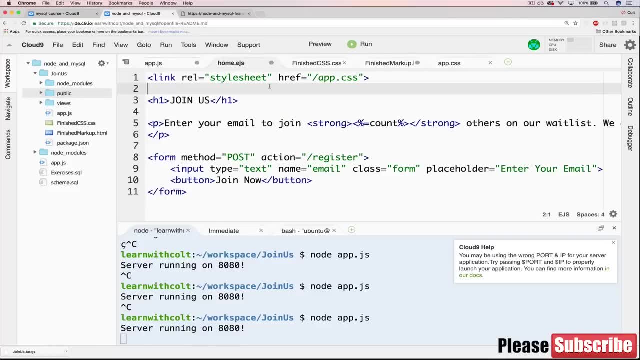 And it's basically saying: take whatever is in the public directory, which is right here, take all the contents and serve them So they're accessible by our views or from our JavaScript. So now, if I should restart the server app, dot CSS is going to be available to this file. 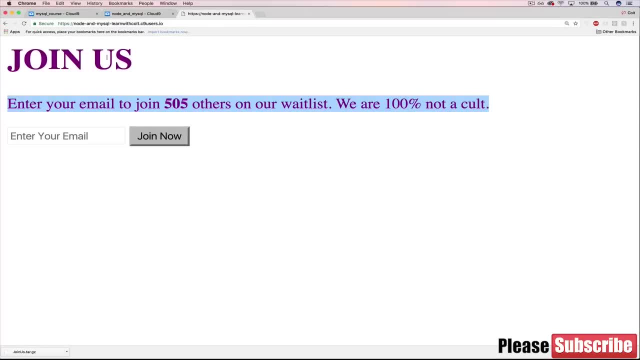 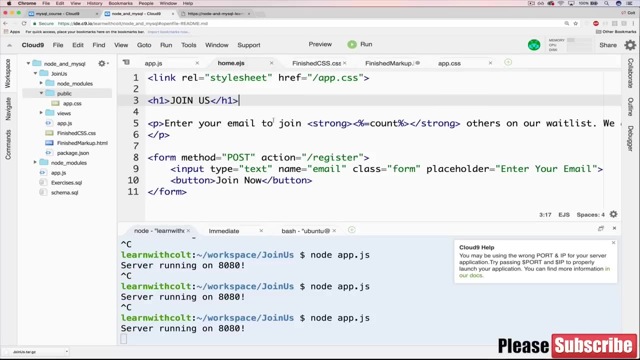 Hopefully, And if we refresh the page, we now have purple text. Okay, so we now have a style sheet connected, And if you had- just as a quick aside- if you had multiple different views here and you wanted them to have the same style sheet, you could use this line in all. 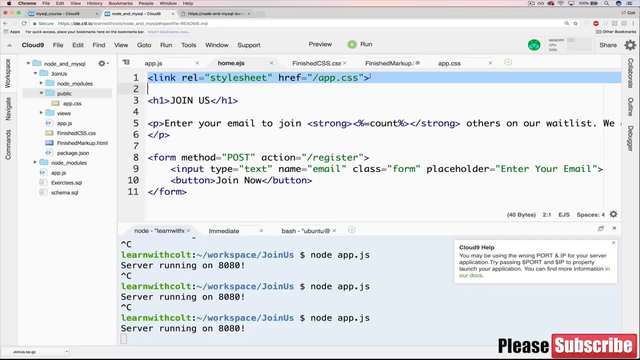 of them, or there's actually a better way, which I'm not going to talk about in this course, called Partials, Where you can basically have code that runs on all of your views, But you could also have a separate style sheet for different views if you wanted to just put them all in public. 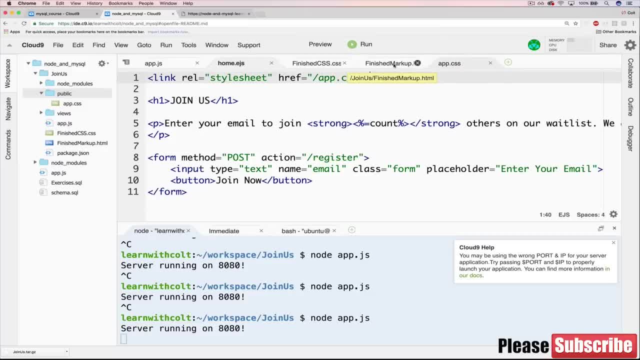 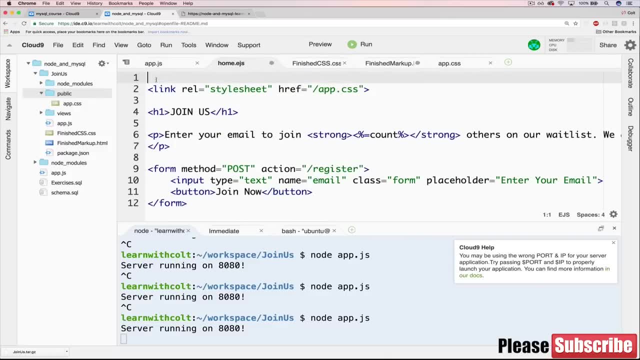 Okay, so that's the first, simplest thing. The next thing you'll notice in the finished markup is there's also a Google API or a Google font that I included, so I'm going to put that in here too. This is for a font called Roboto, pretty common one. 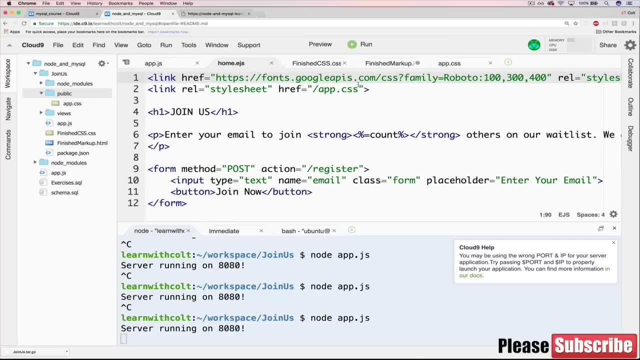 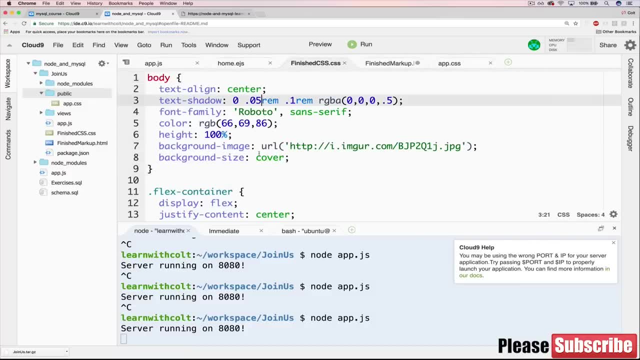 If you're not familiar with Google fonts, really great resource: free fonts that you can use on your own websites, and they look good. So now let's also go back to our finished CSS and let's copy some of this body stuff over, for example, font family. 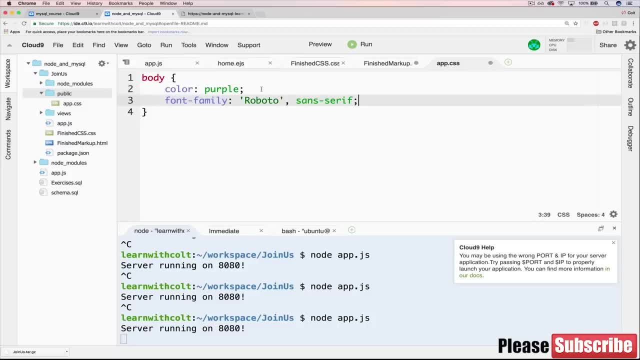 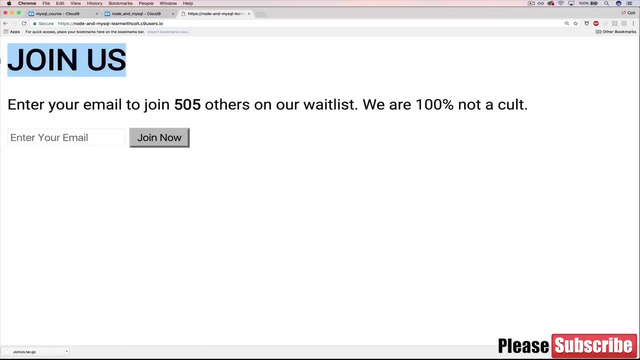 Let's start with that. So we don't want things to be purple, We can get rid of that. But let's change the font so that we now are using that Roboto font. There you go. Our font has changed. slowly getting there. 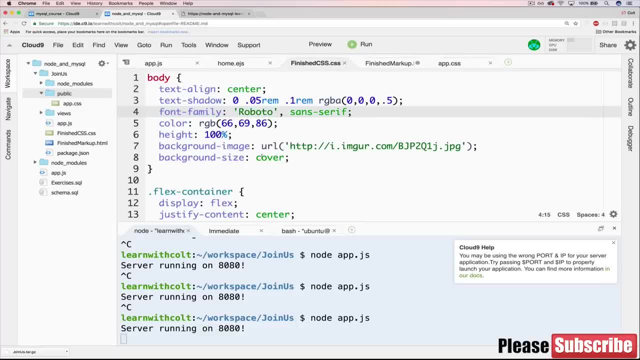 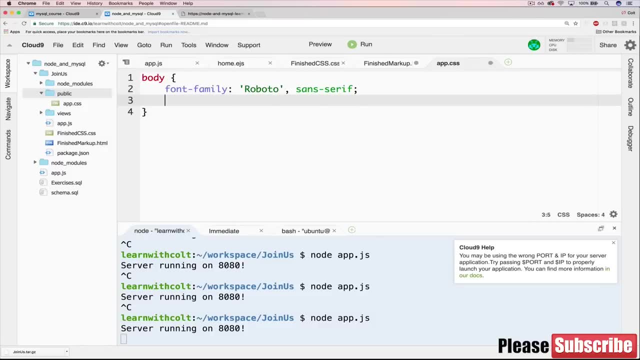 Next thing that we'll do if we go back to our CSS is we'll change the color and the text shadow and the text to line, So I don't need font family again. I'll get rid of that, So line this up. Okay, so this color is like a slightly purpley gray, if I remember. 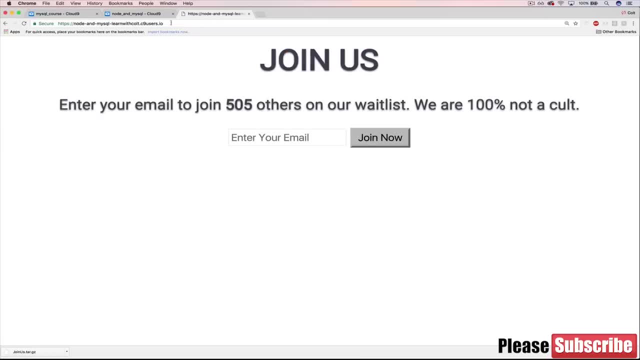 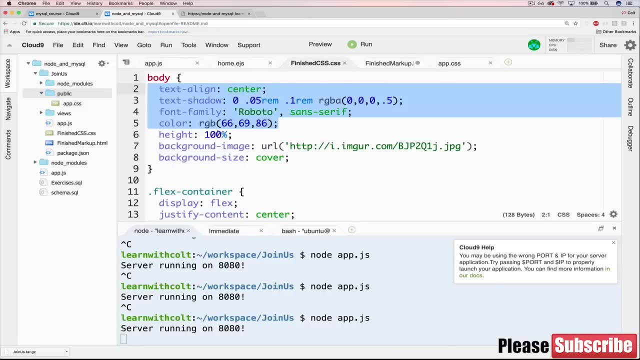 And we've got this slight shadow which I don't know if you could pick up on On the original. we're getting close- Well, that's a lie, but we're getting close to being done with body. Then we've got a couple other things. 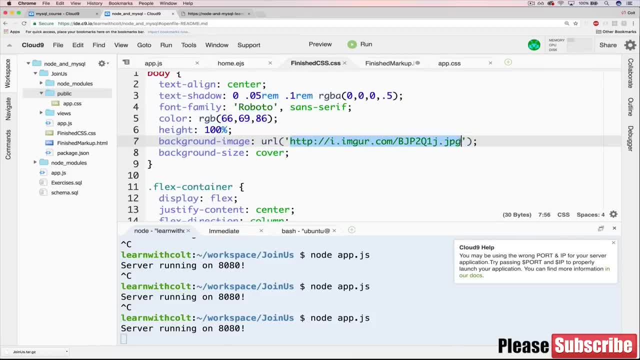 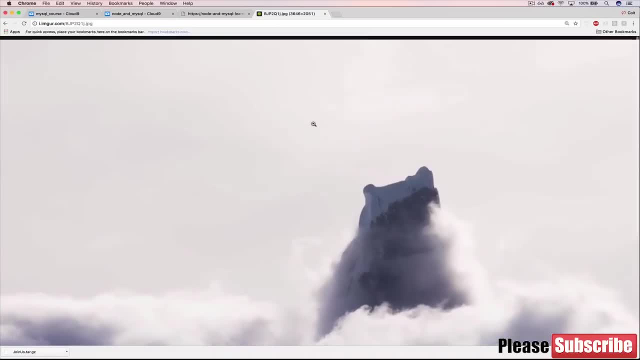 First off is the background image, And if I just show you this image in its entirety, it's a massive image of beautiful mountain in Argentina, down in Patagonia. They took on a backpacking trip. It is called Cerro Torre. 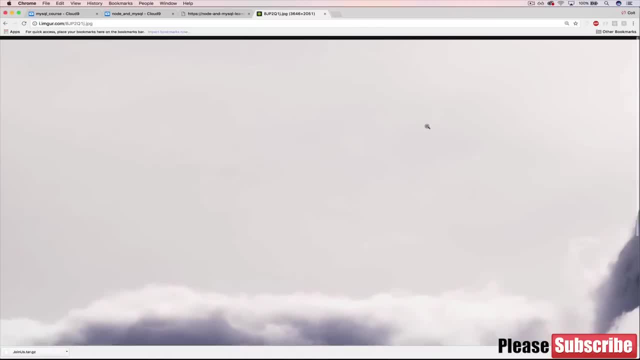 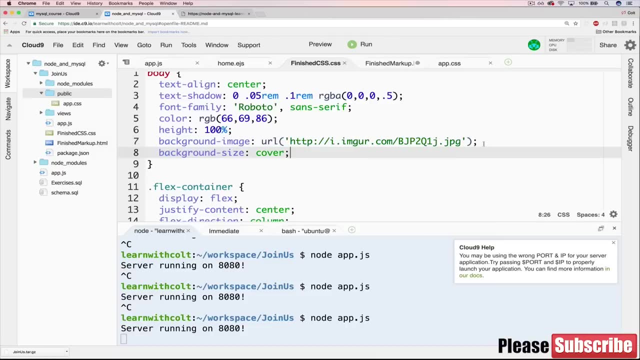 And, yeah, that's my little plug for my photography. Maybe I'll have a photography course one day. So here's this photo that we'll use. We just need the URL and we're setting the body's background image to that photo. Save and refresh. 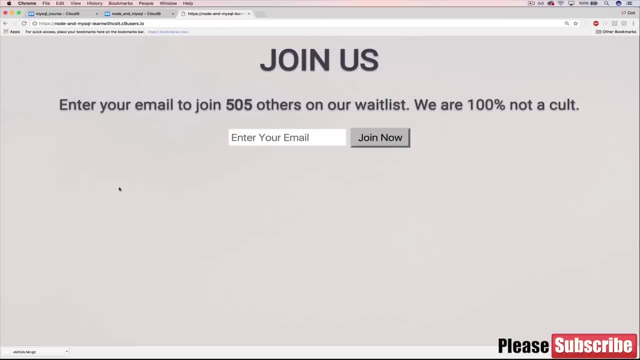 And it worked. but you can see it kind of just looks like a solid color, But it's using the image. It's just so big that it's taking, I don't know, five or six of these screens or more. So that's actually something that, if this 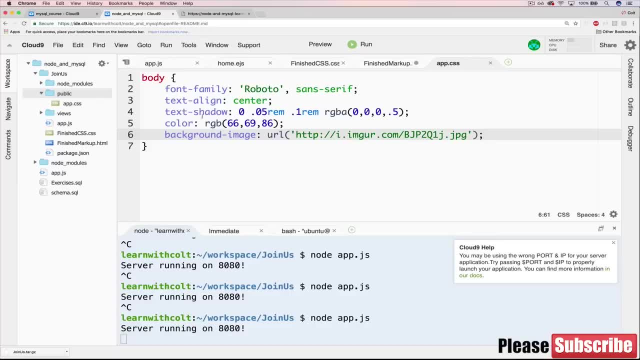 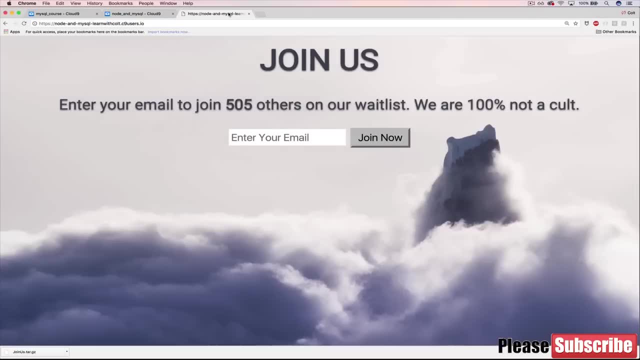 is a real app. it would be good to just use a smaller image So we're not loading such a big image, But what we can do is use background size and set that to be cover, And now it will basically take the image and make sure it covers the entire background. 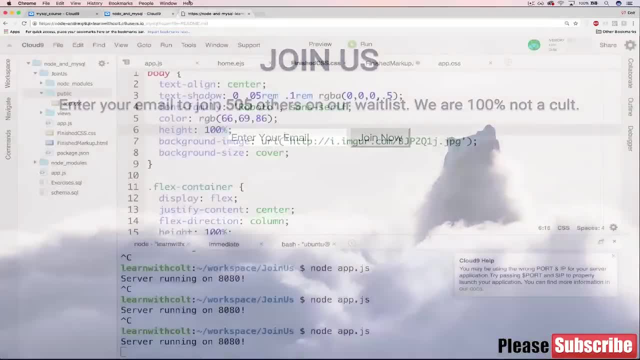 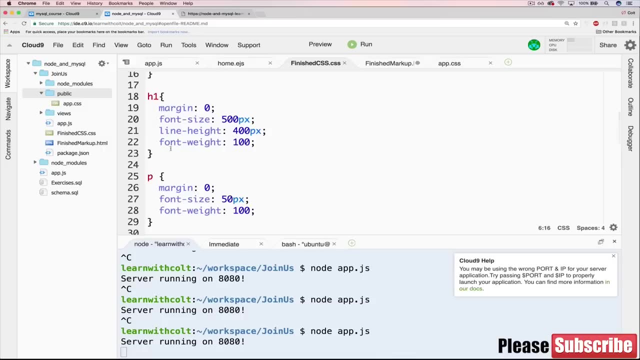 So we've got that. It's getting a little closer. now. The next thing that we can do: if we scroll down, we'll come back to this flex container. We've got our H ones and our paragraphs And, if you notice, I'm setting the font weight to be 100.. 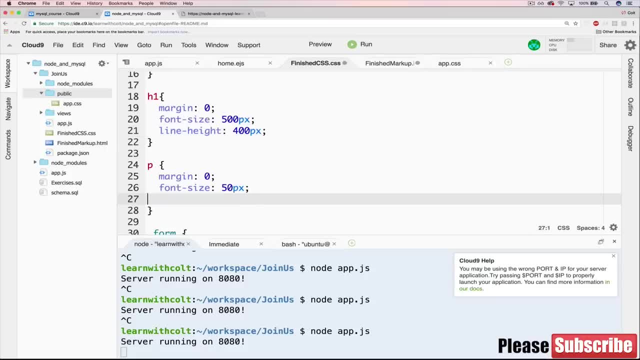 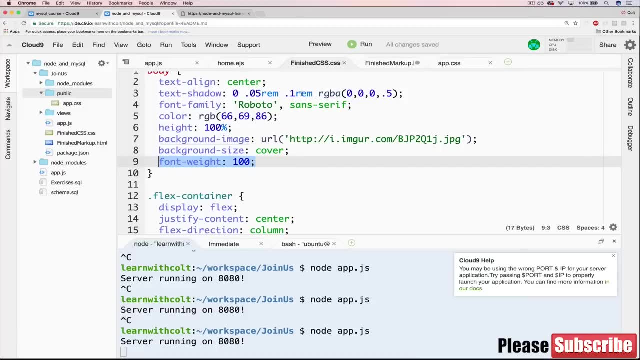 I'm actually going to get rid of that in both of them. There's a better thing that I can do, which is just set the font weight to be 100 in the body, And what that will do is just make our font thinner, so that we get this thinner text. 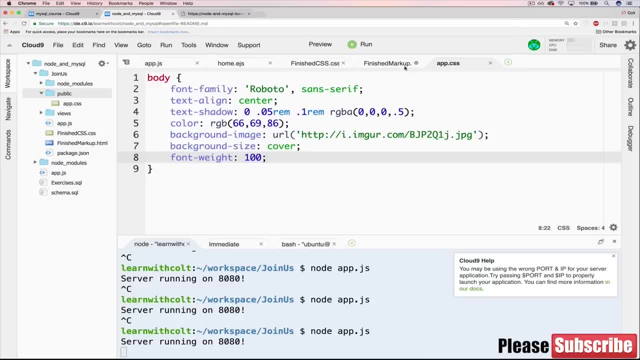 Okay, so we've done that And let's see moving on, let's work on the H one next. So the H one is giant. It's not giant yet, but this- join us- that will be giant in a bit. We've got a couple of things that we're doing. 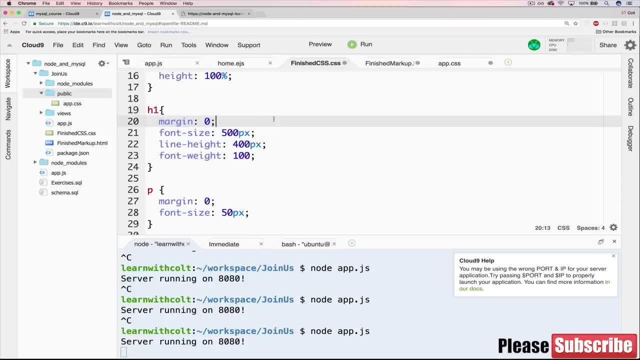 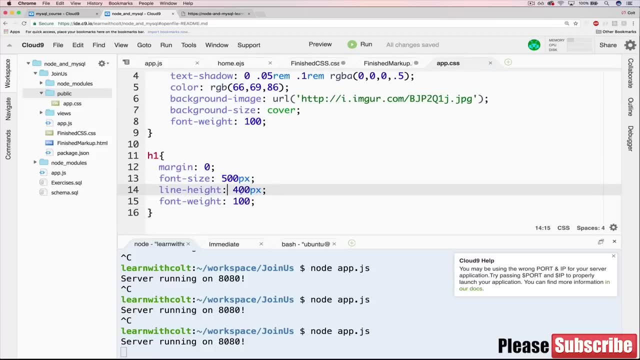 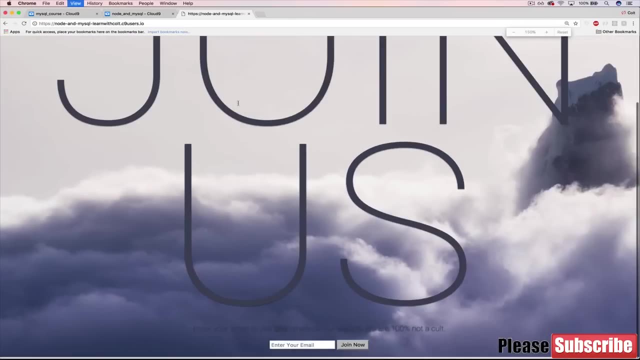 We've got. we're setting- Well, let's just copy it all over margin to be zero. font size: 500 pixels. Line height is 400 pixels. Okay, so it looks massive right now and that's because I'm super zoomed in. 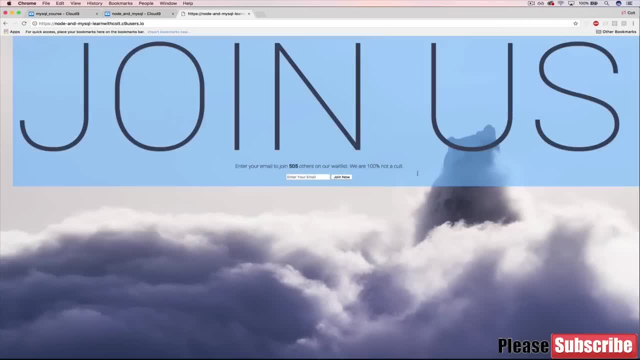 So it's not as massive now. It still is big, but nowhere near as bad. So we've got join us and that's big, looking relatively good. What we want to do, of course, is position it downwards, But I'm going to wait to talk about that. 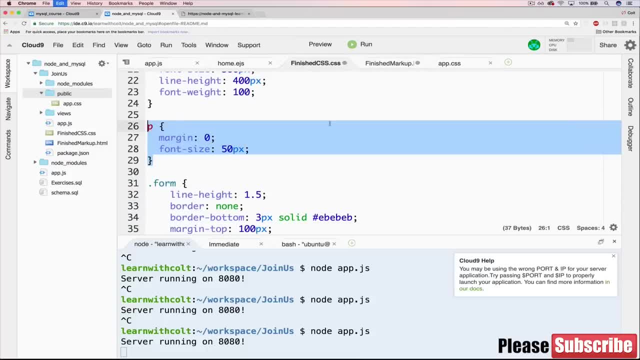 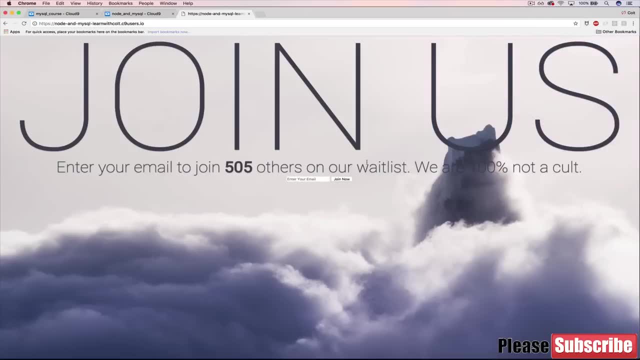 So we'll move on To the next thing. we've got our paragraph that we can style, And really all we're doing for the paragraph is changing the font size, So this here gets bigger. Then, after that, we're onto the form and the button. 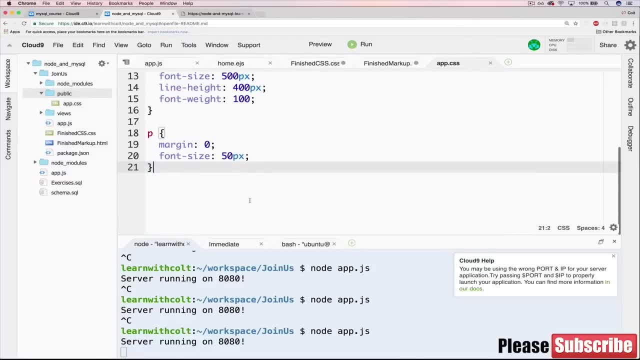 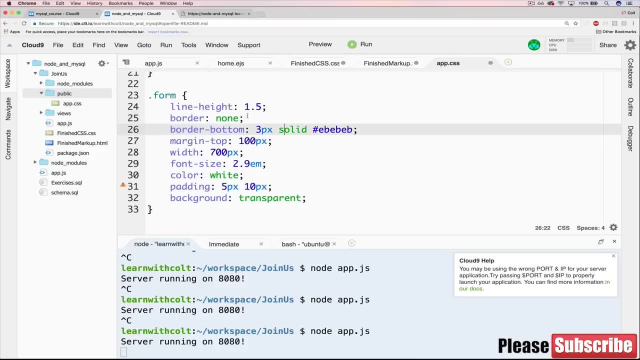 So I'll just copy everything from the form to start, and I'm going to comment things on and off as we go. Okay, so look at our form right now. Quite ugly. Let's start by taking a look at. Well, line height is simple, but border none. 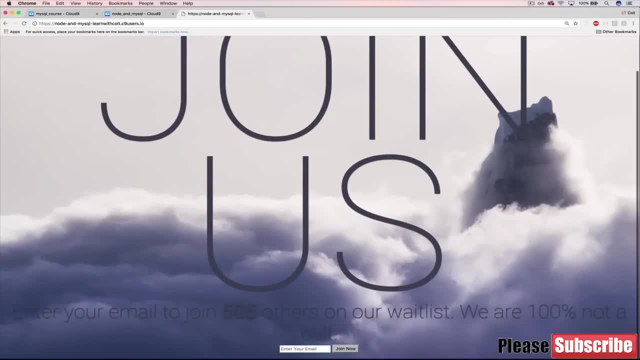 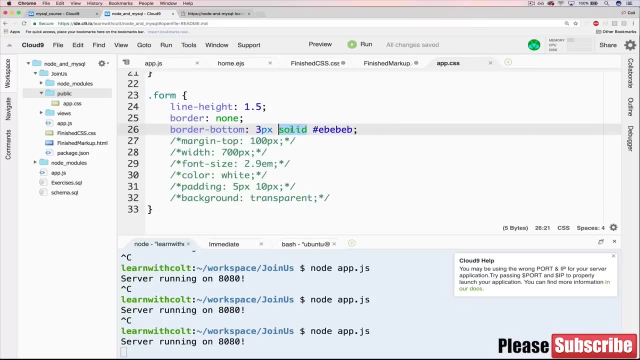 What that will do if you will make it bigger. If you look at the form down here as I refresh, I don't know if you could see, but a border went away- the default border- Then what I'm doing is adding in a line at the bottom. 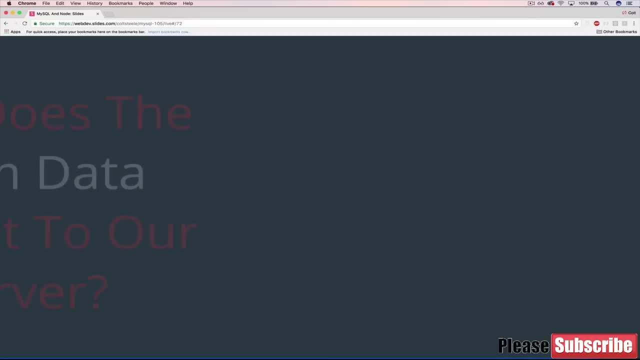 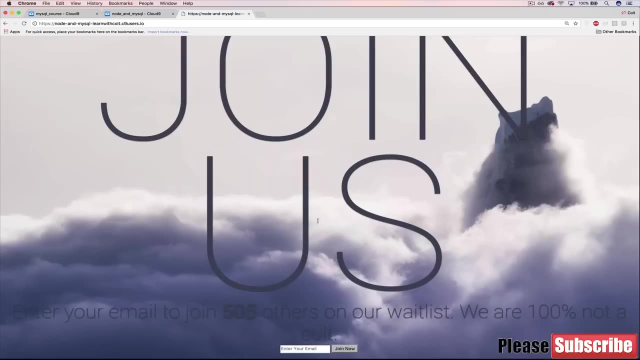 And actually what will make this easier is if I just show you the finished app Just a moment. Here you go, See, we have that white line running underneath. So that's what I just added in. It's very hard to tell because we still have the rest of the form there. 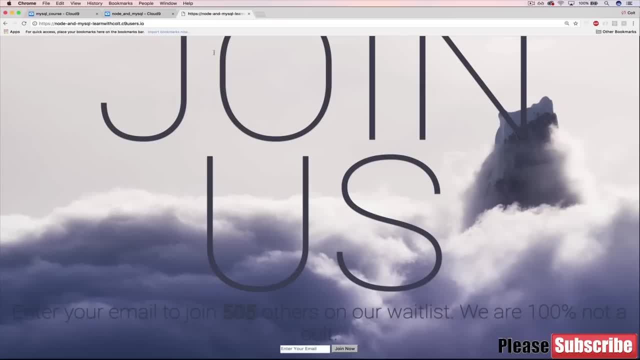 So the next thing: let's make the background transparent. Okay, so it's easier to see, even though it's very small on the screen right now. Now there's no white background And a couple other things. I made the fonts. Oops, get rid of that. 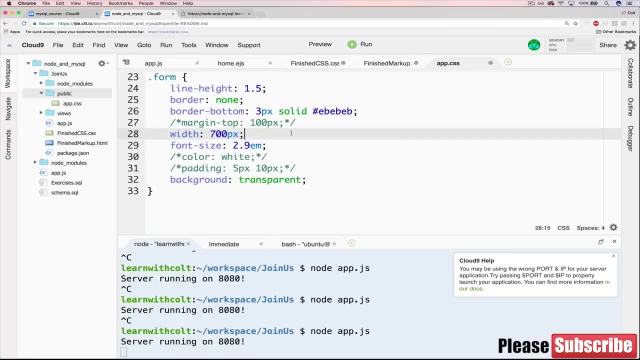 Made the font size bigger, Made the form or the input itself bigger, and then included a margin, a color and some padding. Also, I'm using a class here. It could also just call this input, But what's being styled is not the form itself. 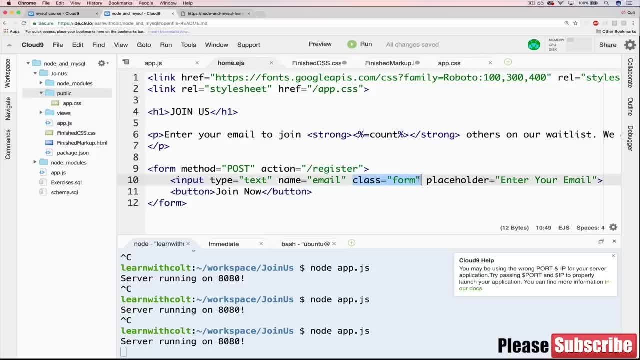 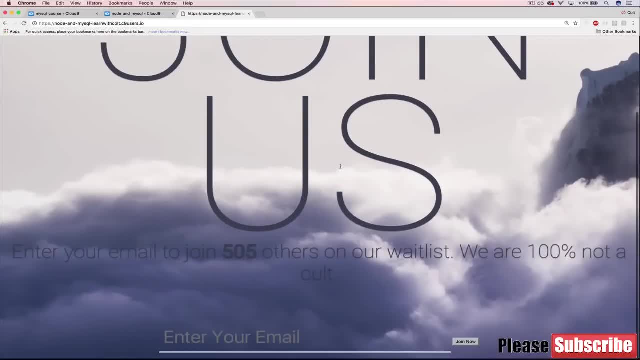 But if you look here, we have a class equals form, So it's the input right here. Refresh now and we're getting closer. Let's go back to 100.. One thing that you may notice is, when I click here, I get this annoying focus effect. 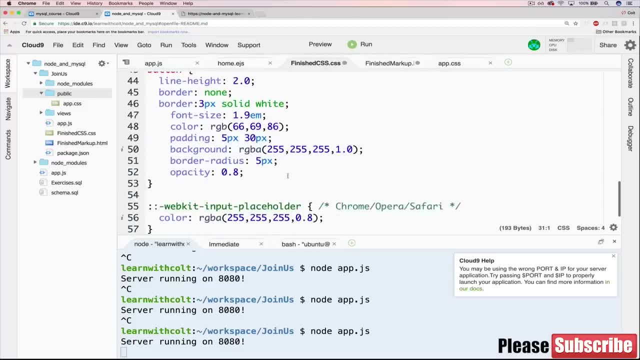 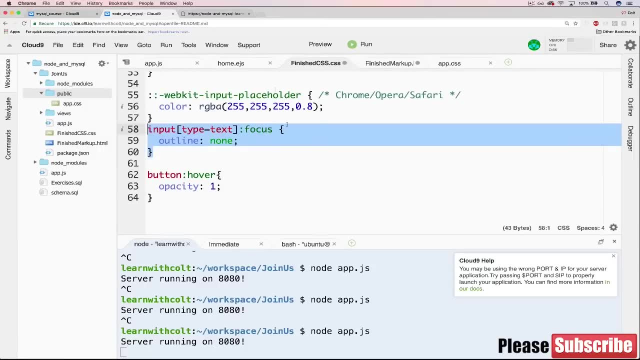 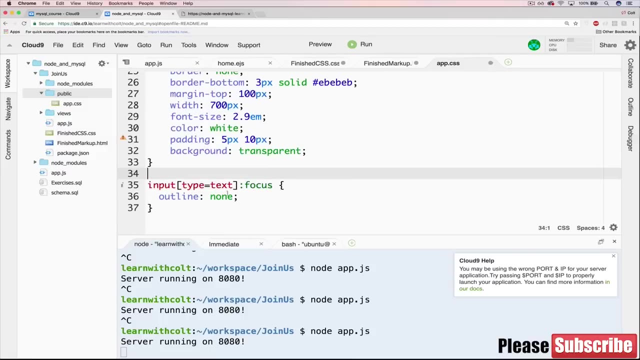 We can get rid of that with CSS, which, if we go to the bottom, we've got this input Type equals text focus, And what this will do is say, when an input with type equal text is focused when someone clicks on it, there should be no outline. 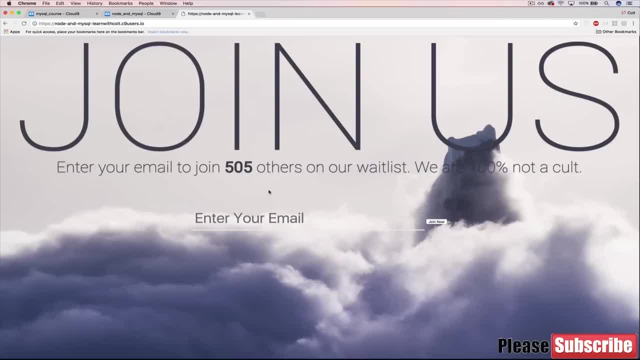 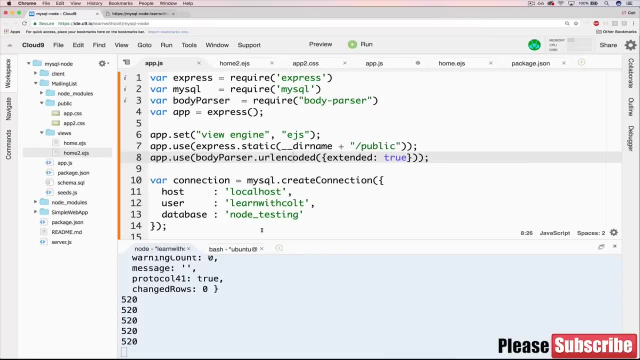 So if we save now and try it, I don't get that weird outline. Also, if you notice, I have the text white here. I don't know why I decided to do that. This is placeholder text is what this is. So as soon as they start typing, it turns white. 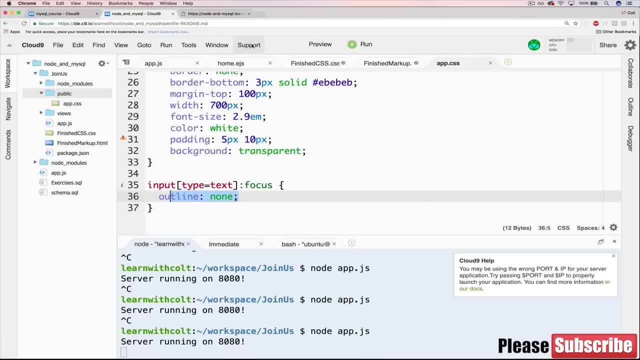 But the placeholder is dark. To change placeholder text is a bit annoying. I'm not going to even bother spending much time on what this is, But if you notice, there's this fancy. basically it's a CSS three browser specific way of doing this, where we're targeting the input placeholder text. 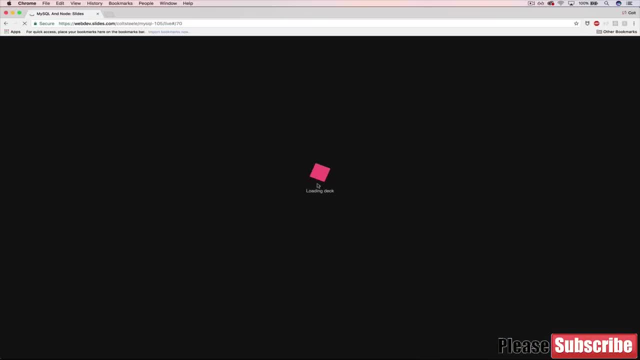 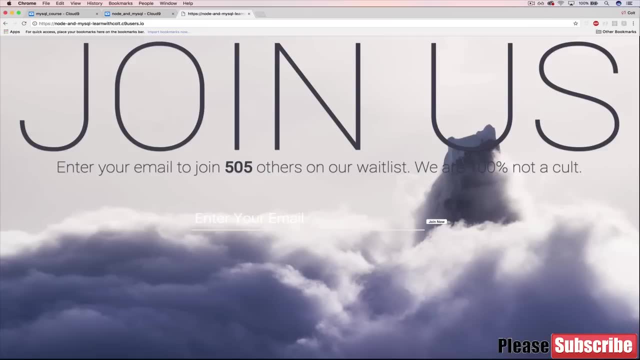 And I'm setting the color to be slightly see through. So now if I do it- oh, that's not what I wanted to refresh. Now if I do it, it's slightly transparent, but I start typing, There we go, Okay. 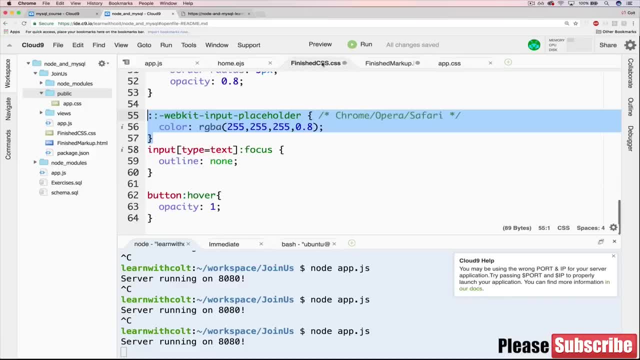 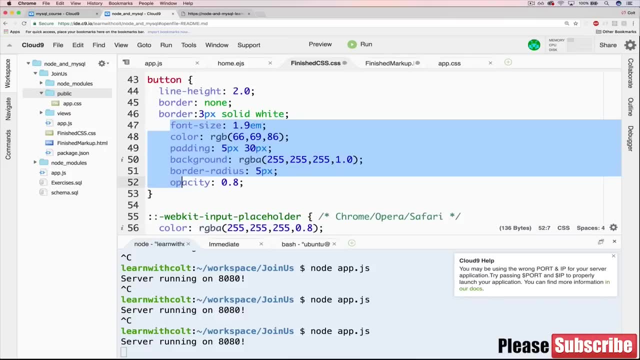 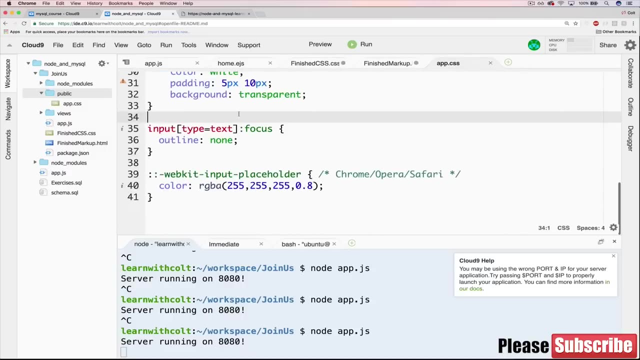 Moving on, Moving along. That takes care of our form for the most part. Now we've got the button. The button is pretty straightforward. Let me format this a little better. I'll just copy it all over And save mainly what I'm doing to actually. 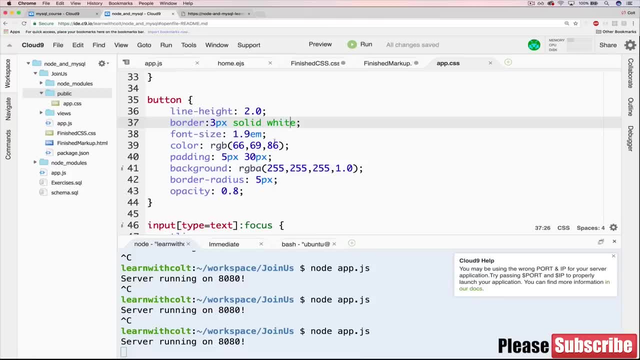 get rid of this is adding in a three pixel solid border. Then I'm making the font size bigger, I'm making the color, I'm changing the color, Adding some padding, adding a background color, And then so the color here is referring to the text. 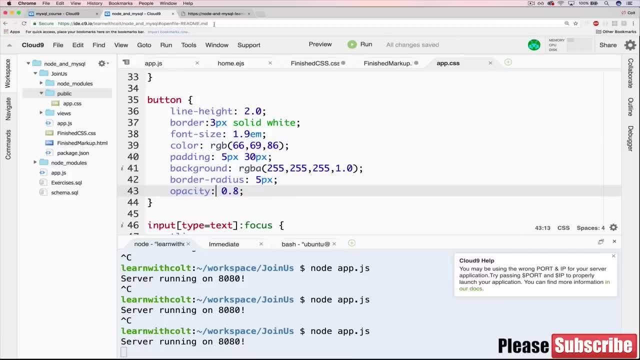 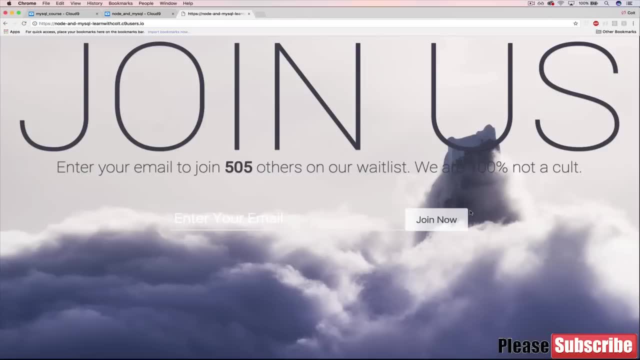 a border radius to make it rounded, and then making it slightly see through again, So you can see that change is made. I'm not a designer, so I'm sure there are many better ways, things we could do to just make this look better. 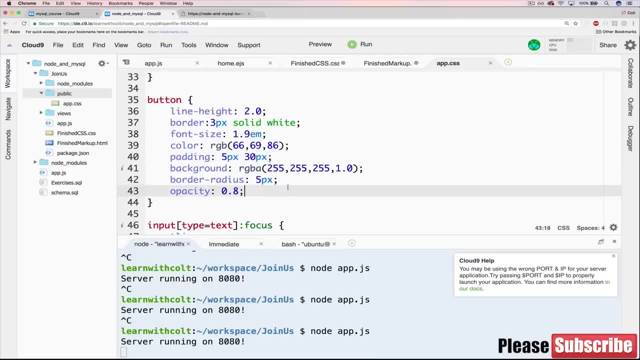 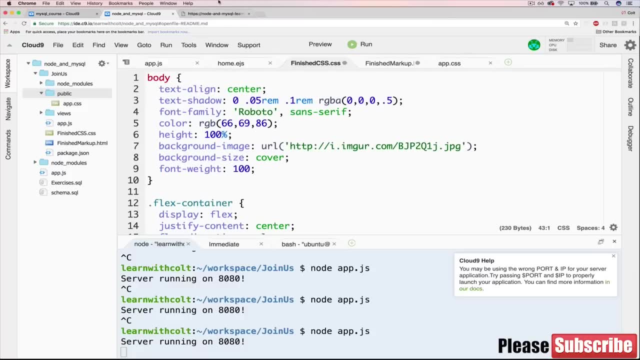 I'm not terribly happy with it, but it's good enough for my SQL course. So that's pretty much it for the button, which then leaves us with basically positioning things, Formatting them. How do we get this to be centered vertically, roughly vertically, in? 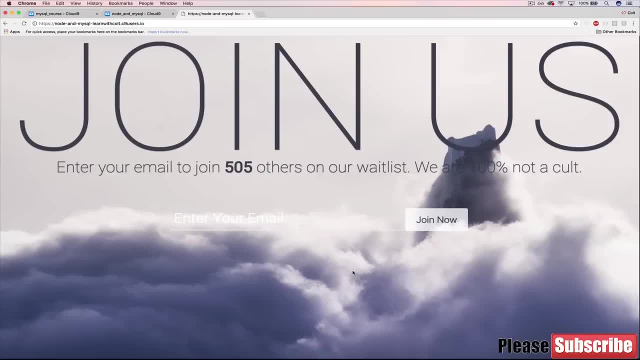 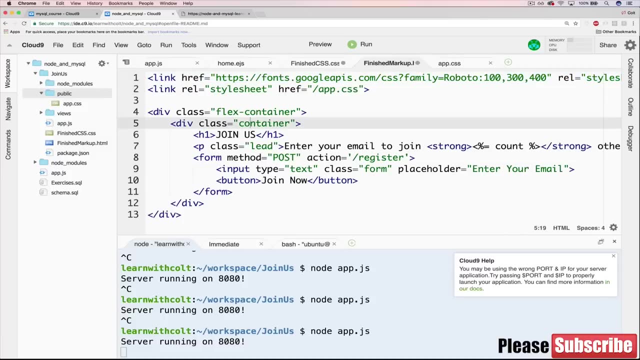 the page, which is what we did here, what I did here, And it's not too bad. All that we need to do is change our markup a little bit. So we've got basically two divs that everything is wrapped in. The first one contains everything. 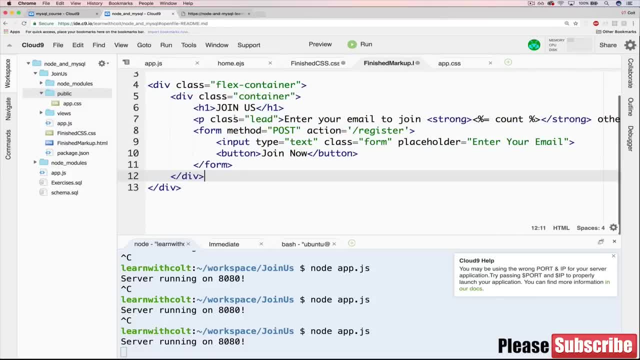 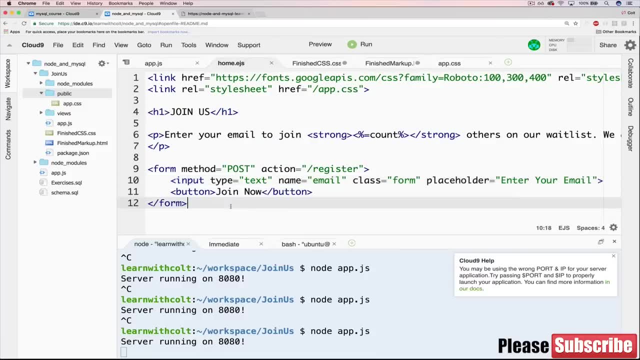 And then there's a second one that also wraps around everything. The first one is called Flex container and the second one give a class of container. I'll just copy this and paste it over into home EJS, But it's the same content. we've got to join us. 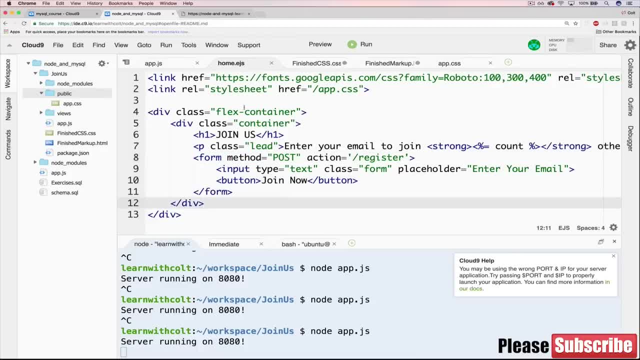 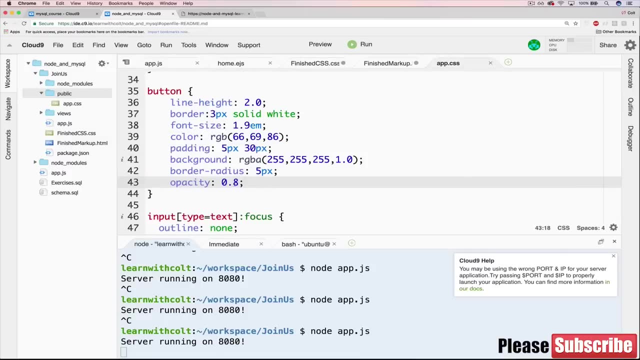 We've got our paragraph, our form, But now we also have these two divs on its own. I refresh. Nothing changes, However, if we add in this little bit of CSS here, But this will do its help position things vertically, so we can put this and we can. 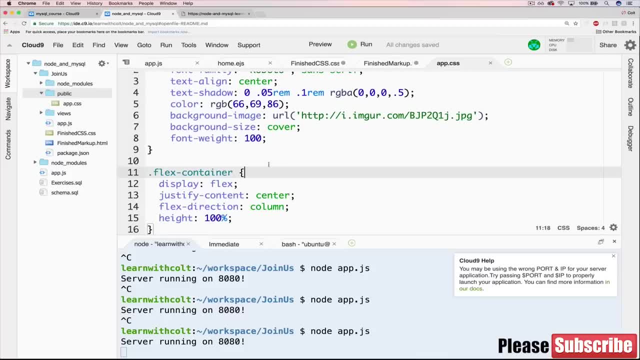 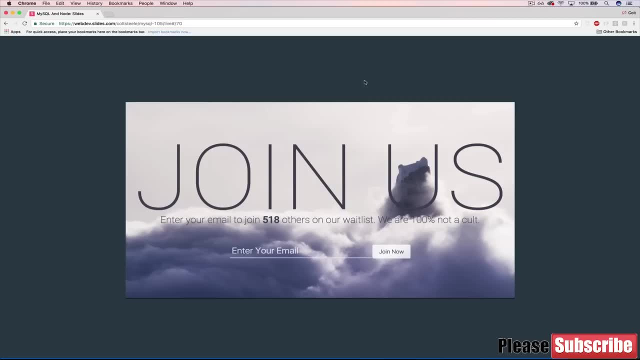 put it wherever we want, but I'll put it towards the top. Now, if I save and refresh the page Now, we've got everything vertically centered. So this isn't a course on CSS, so it's not a course on things like flex box. 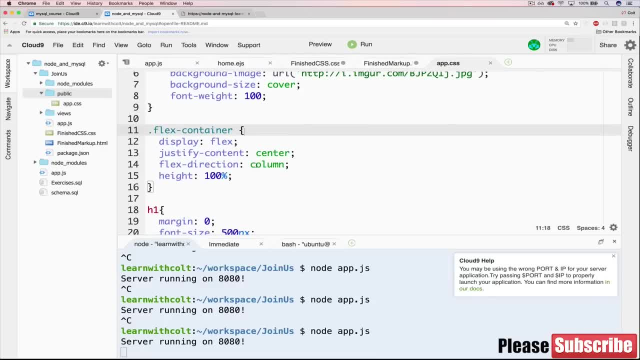 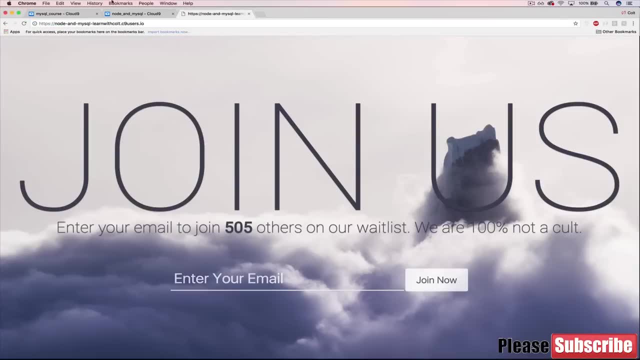 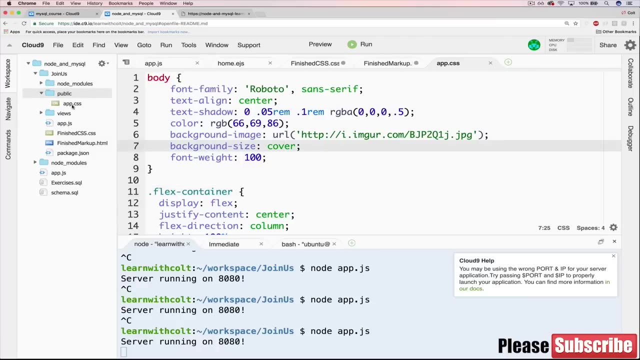 or positioning or what these fields do, but this is a nice and easy way to position things- well- relatively easy- And so we're basically done here, just to review what we did. The first thing that we did was to allow or to set up our app so that it was serving a public directory, which was this fancy? 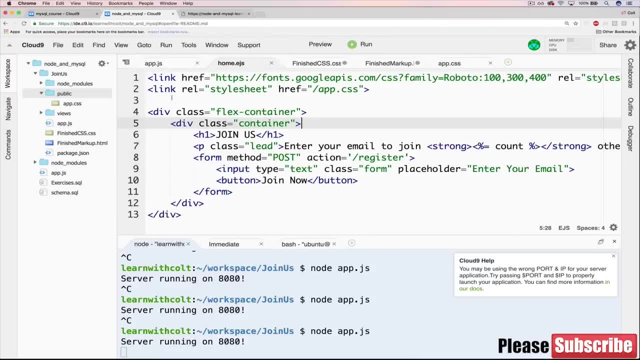 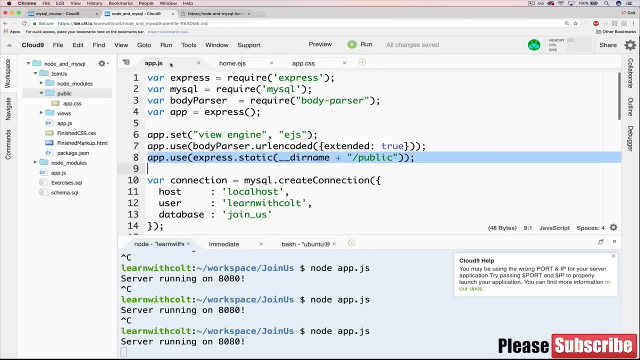 line here. everything inside the public directory is now available in our views. So what I'm going to do, I'm actually going to close down our CSS and markup So we just focus on what we actually have. So then, in our home, that EJS. 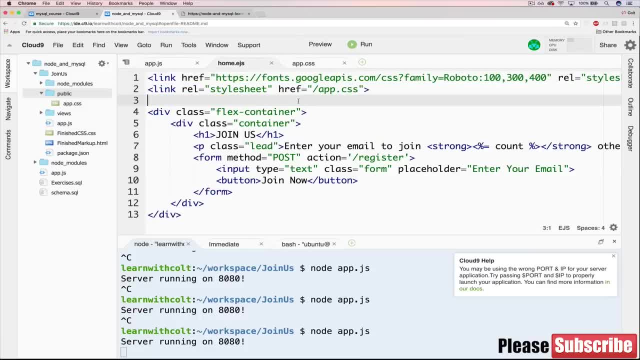 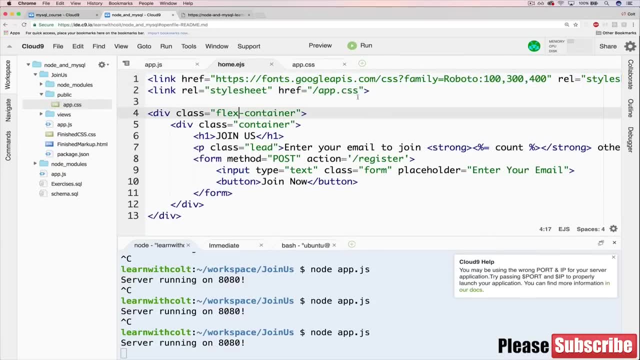 we can link to app dot CSS. We do need that slash And it's referring to this app dot CSS there. OK, so then, aside from that, we added a font And then in our app dot CSS, we added a bunch of styles which we mainly copy. 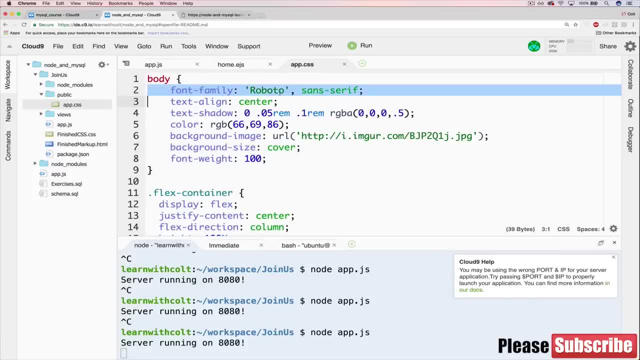 and pasted. It's not the point of this course, but things like changing the font, adding a text shadow, changing colors, adding the background image, changing the background image size, how it's positioned or how it's sized, taking up the whole screen but not overwhelming it. 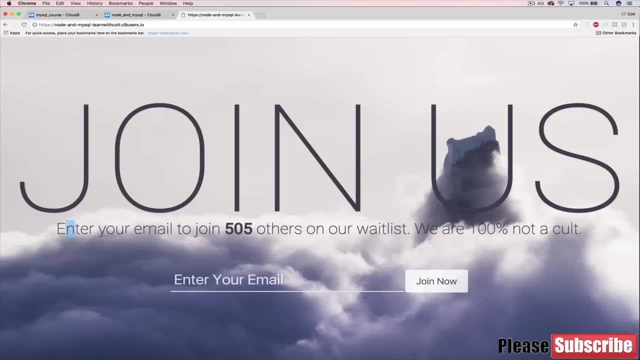 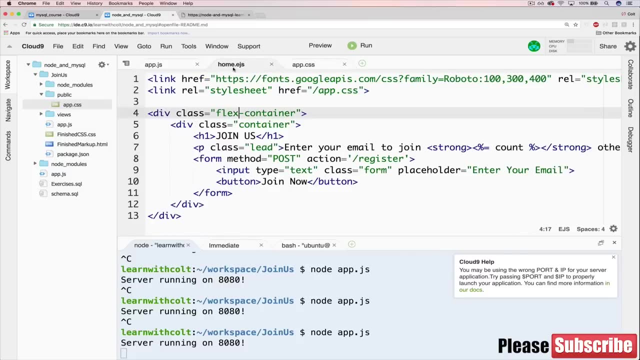 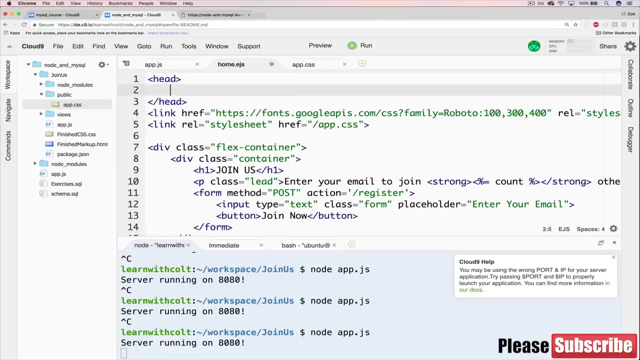 And then also the font weight, making our font lighter weight. Then we've got our form and our button that we formatted, and then also we position things using these two divs and styling those. One thing that we could do to make this a little bit more kosher is to add a head and a body to it. 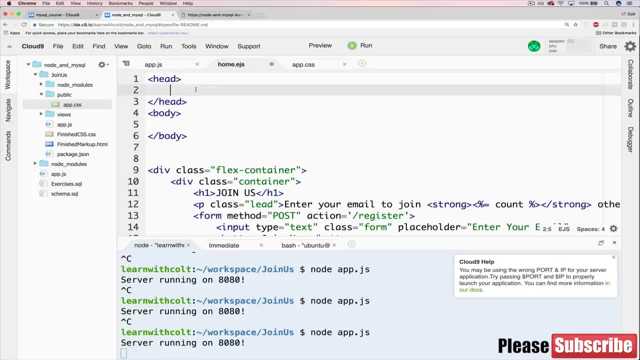 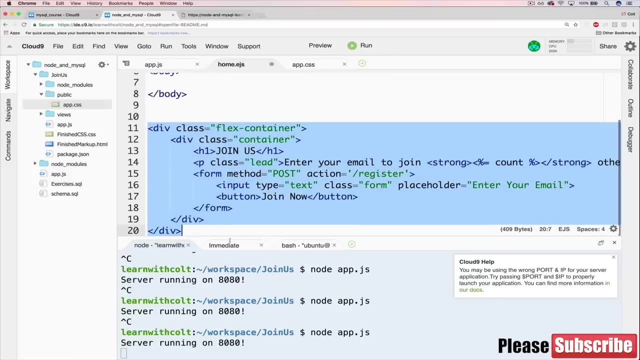 So if you're familiar with HTML, you've probably been asking why we haven't done this, You don't? I mean, we should have it there, but we don't have to have it. A browser will add it automatically, But it's definitely an improvement. 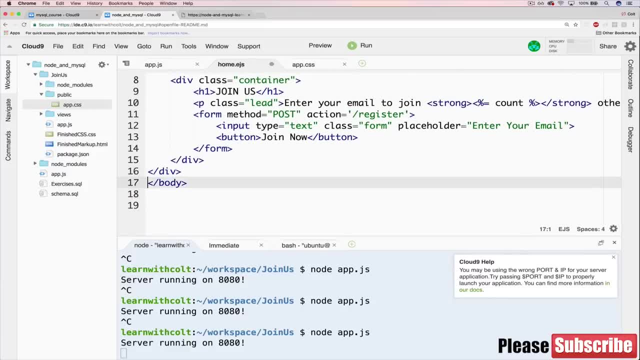 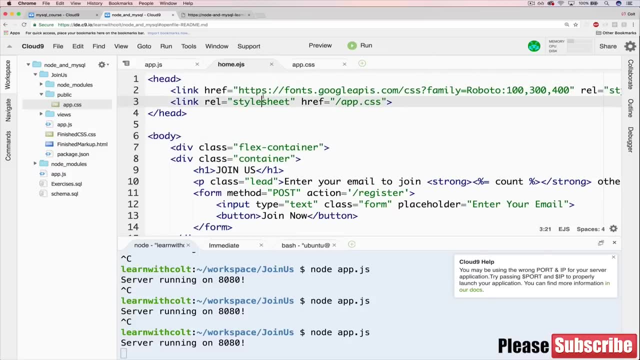 to follow convention to do, to not rely on a browser to do that for us. So now we've got a nice, officially formatted kosher. home that EJS file and just double check that it still works All right. And let's make sure our form still works. 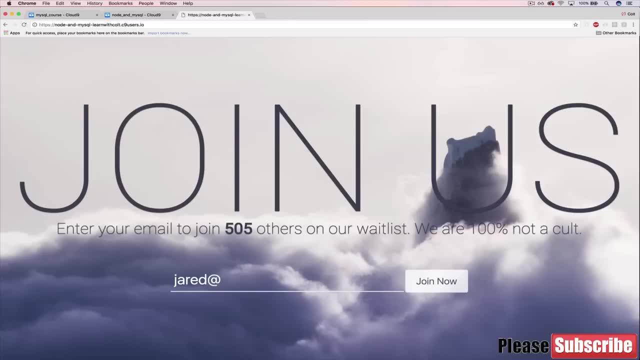 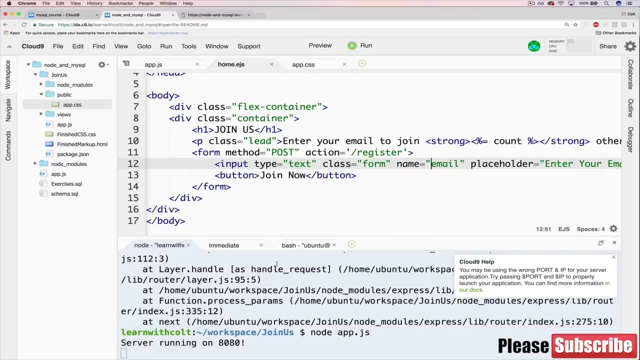 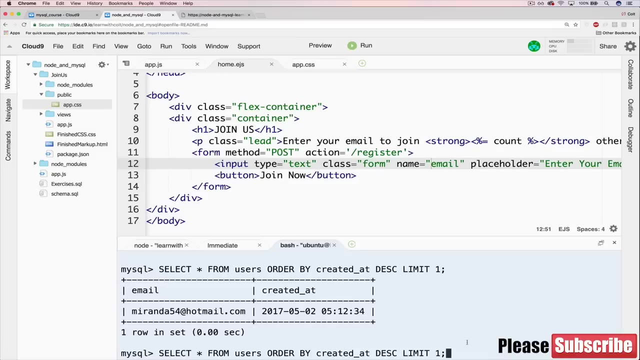 No reason it shouldn't. But let's add in a Jared at Gmail dot com and we hit join now And we see we've gone up to 506 now and we could go over to my SQL. run the same query: select star from users order by created at descending this time limit one. 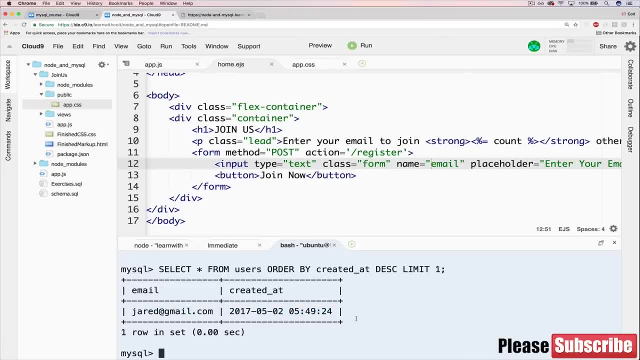 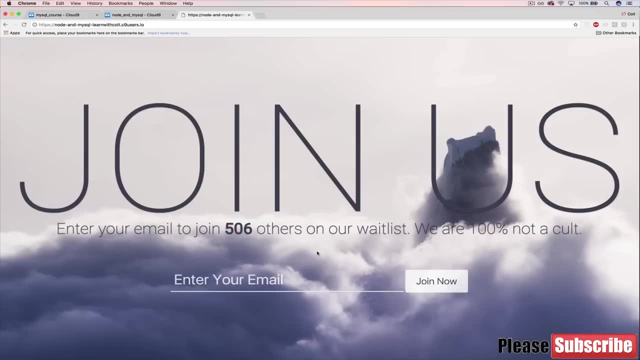 And we get Jared at Gmail And we get the correct timestamp And we're officially done with this app. So if you wanted to, of course you could change, you could create a second page to redirect to that said thank you or congratulations, or you could restyle this or you could collect more information. 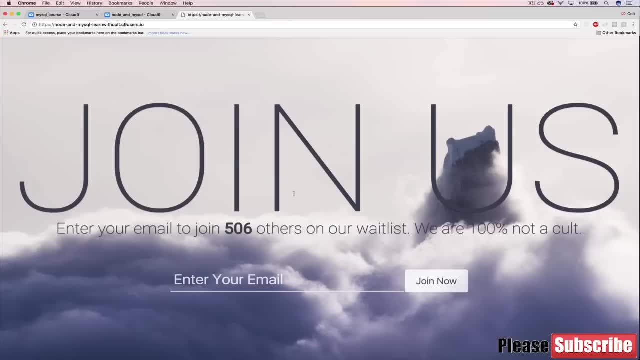 If you wanted a challenge instead of just an email, collect a name or a birthday or a phone number. That's more useful than an email. People will give it away at least. So this was a lot, two sections just to make this work. 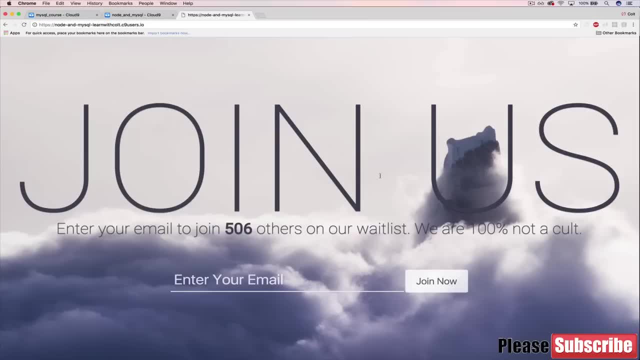 Although, if we really think about it, the bulk of it was introducing things like node and NPM and and my SQL package and CSS and HTML EJS. So much groundwork for an app for a simple web app. But the my SQL part was super easy. 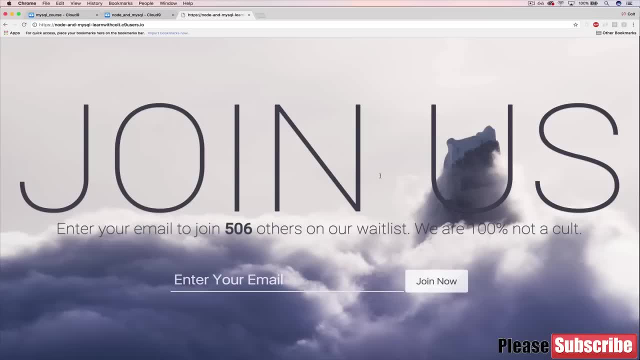 Hopefully you know creating a table and inserting a single thing or selecting account- stuff that we've been doing for a long time in this course, so hopefully you feel good about that. And this was more of just a high level survey of creating an app. 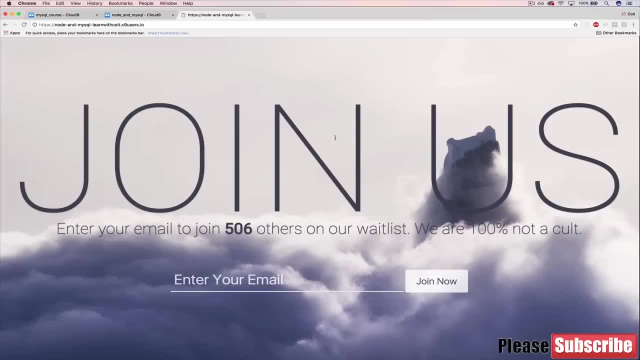 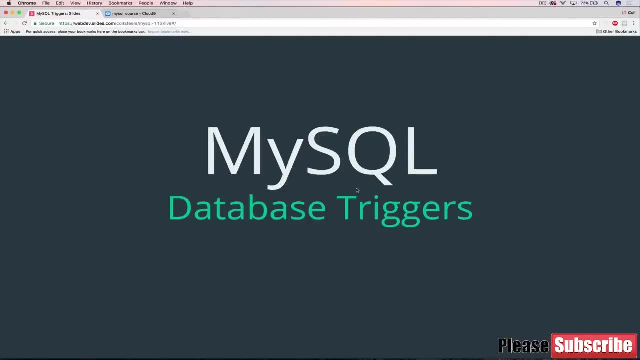 But I want you to feel like you know you leave this course making something, even if it is simple. But you've now seen how all the parts fit together. All righty, Welcome back. So this is a new section, not just to you. 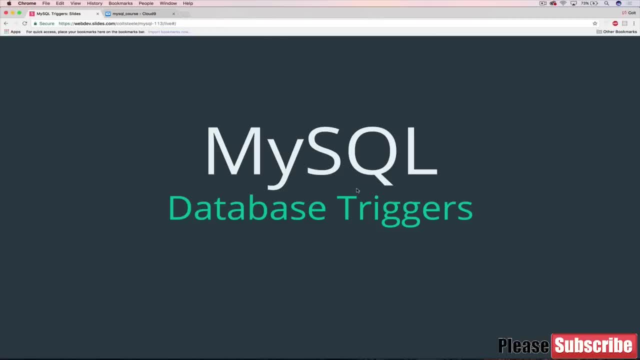 Obviously, it's new if you're watching this, but new to the course itself. I added this. It's basically a month right now since I published the course And I'm adding it because a lot of people have been requesting this topic. 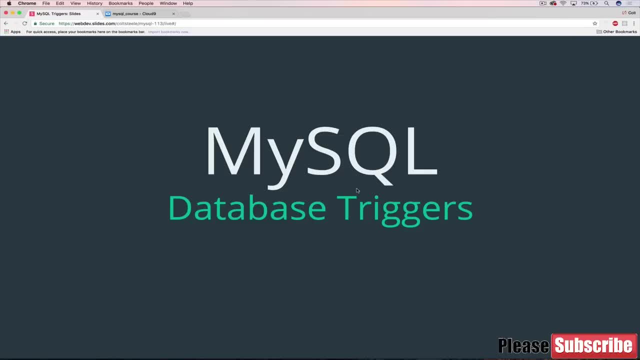 There's been a bunch of comments and people have been asking about this, So I decided to add it, And that topic is database triggers. So if you're worried about it, if it seems super advanced, it's actually much simpler than learning some of the earlier topics. 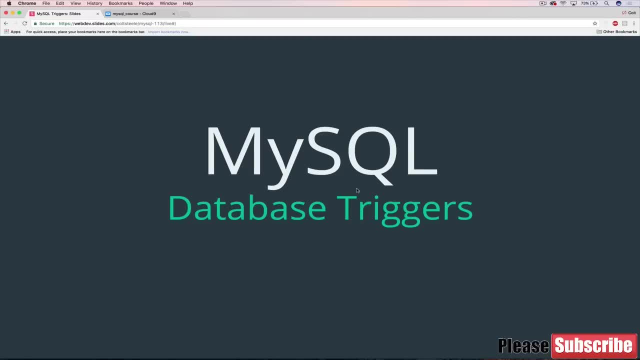 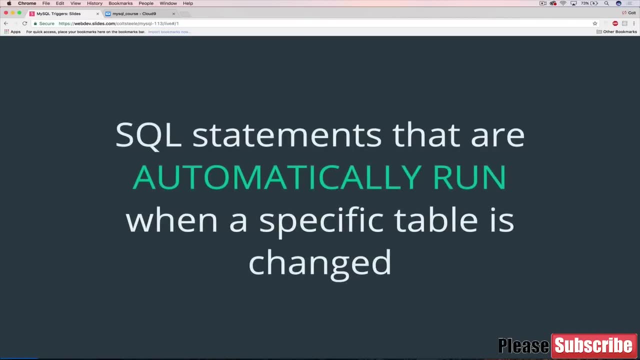 Things like joins are much more complicated conceptually, So this is nice and easy. There's just a little bit of new syntax we need to talk about. But before we get there, let's talk about what the heck it is. What are database triggers? 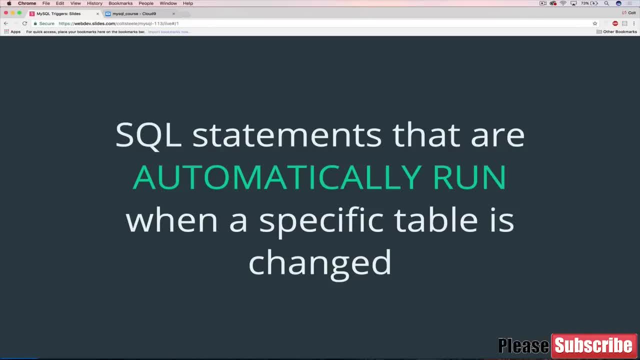 They're just SQL statements, bits of code that are automatically run when something happens, when an event triggers them, so when a specific table is changed. So this is actually really, really useful In certain situations. So I should start off by saying this is: 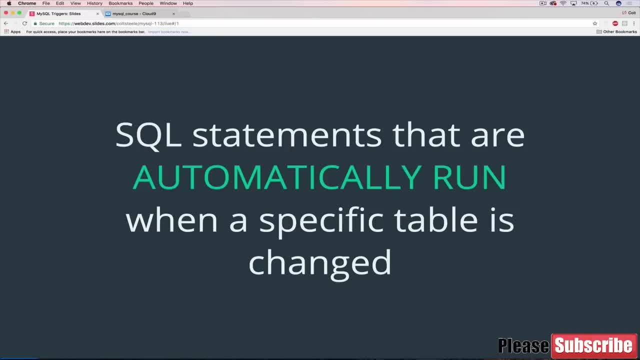 not something that you'll be using all the time, even in a big. you know, if you work at a big company with a big production database, you're not going to have a bunch of triggers, You're not going to be writing this type of code often. 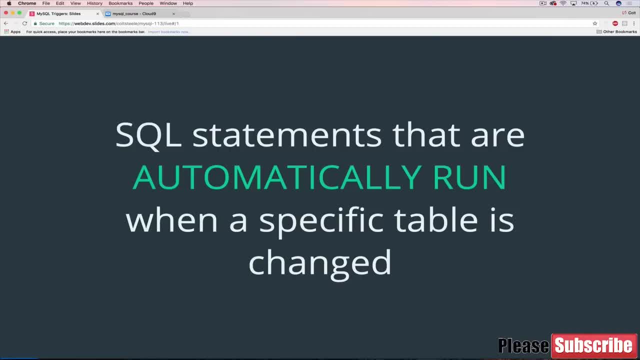 So it's not central to using MySQL in any way, But it's a nice thing to know how to do And when you do need it, it's really nice to have. So again, it's basically SQL code that will automatically run when they're triggered by certain events. 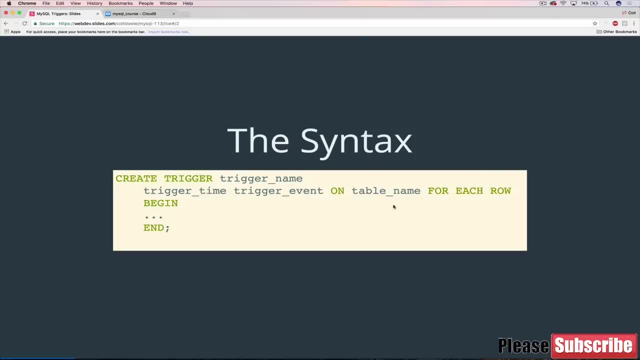 So here's the syntax. It's not going to make a bunch of sense just looking at it like this, But here's the rough pattern. So there's this new bit of code: create trigger, and then we provide a name, And the name is not all that important. 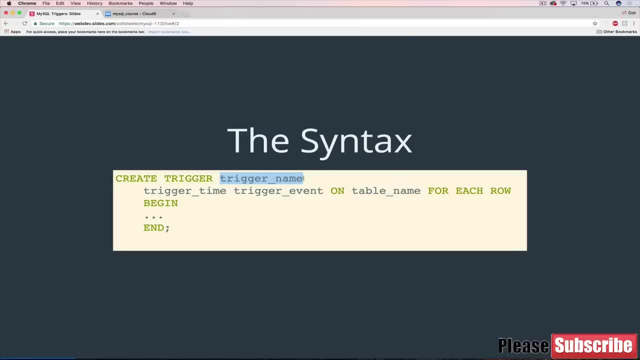 It's really for your purposes, for referring back to it Or if you're trying to remove that trigger later on. But as always, you want to give it something meaningful. But then we have three really important components: The trigger time, the trigger event on and then the table name. 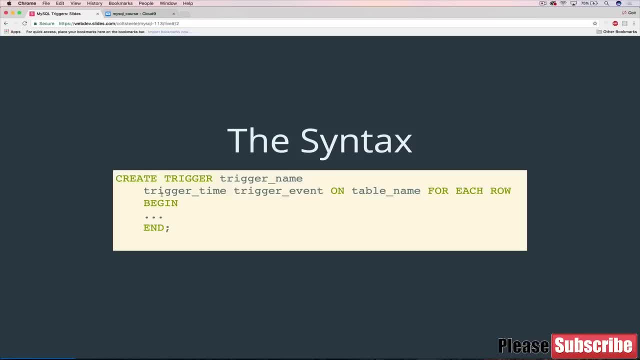 And then the syntax for each row: begin and end. So we'll talk about the syntax a bunch more, We'll write some code, But let's dive into these three things: Trigger, time, trigger, event and table name. Hopefully it will make a bit more sense. 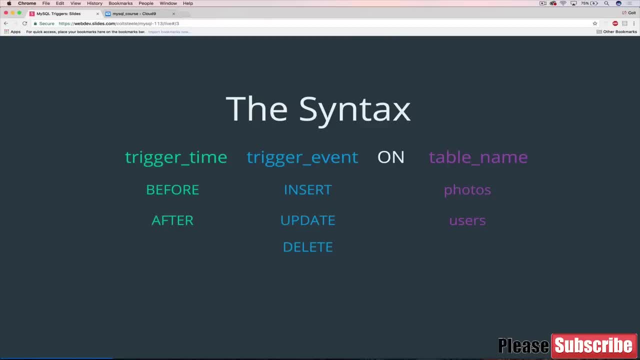 So, as I said, these triggers run code when a particular event happens, when a table is changed, And these three components are very important to that. So the first one is the trigger time, And there's only two choices, before and after. So do you want this code to run before something happens? 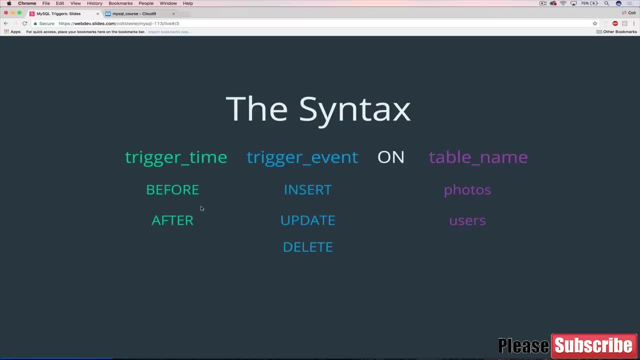 Let's say, An insert. Do you want this code that you have to run before you insert or after an insert? Then, moving on, we have trigger event. There are three choices here, So three changes that can trigger this code to run. 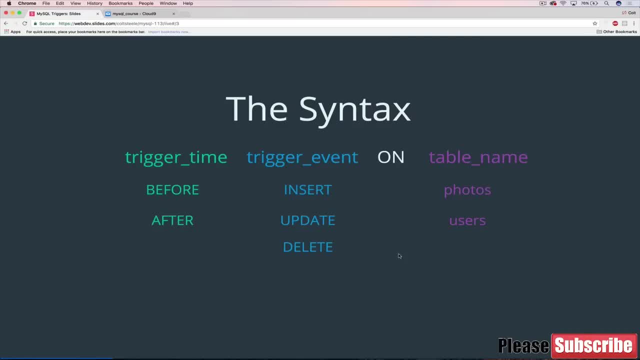 We have an insert, an update and a delete, So you can run some code right before something is inserted into a specific table, or you can run code right after something is deleted, and I'll show both of those examples, actually, as well as update. 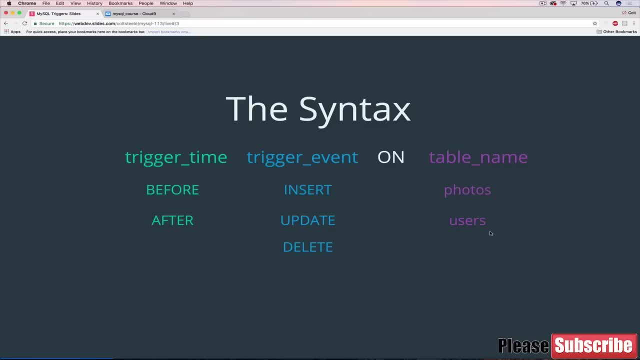 And then table name has basically infinite choices. It's just the name of a table that exists in your database. So we could run some code before you insert into photos or immediately after updating the users table. So whenever that happens, when any single item in the users table is, 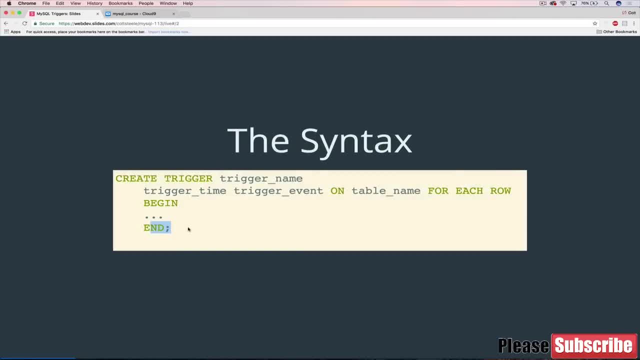 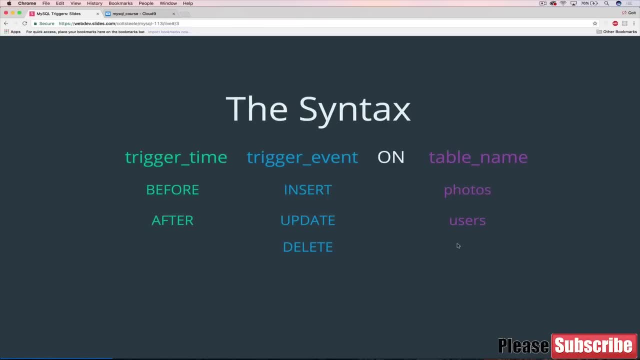 updated whatever code that we have between the begin and end- And there's a lot of new syntax, I know, So don't panic, We're going to get to that in just a bit- But whatever code you have there will automatically be executed right after a successful update on any item in the users. 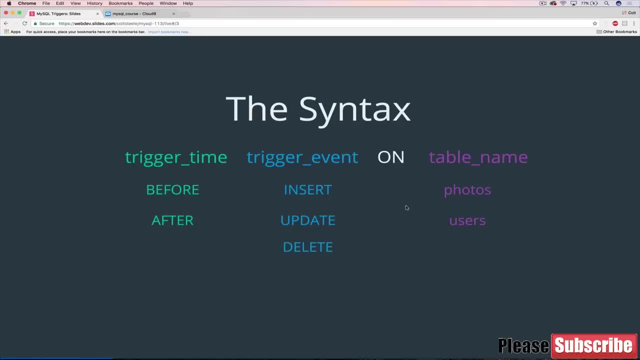 table, And we could do the same thing for delete or insert. So the last thing I'll talk about in this quick intro video is: what kind of things would you do with this? And there's really a couple of categories. The first has to do with validating data. 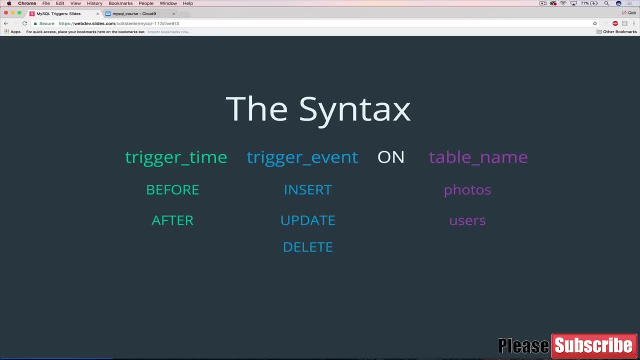 And this is a bit controversial, in my opinion as well, And I'm not just saying other people think it is, but I actually don't think this is the best use of triggers. but what you could do is enforce specific things on your data. 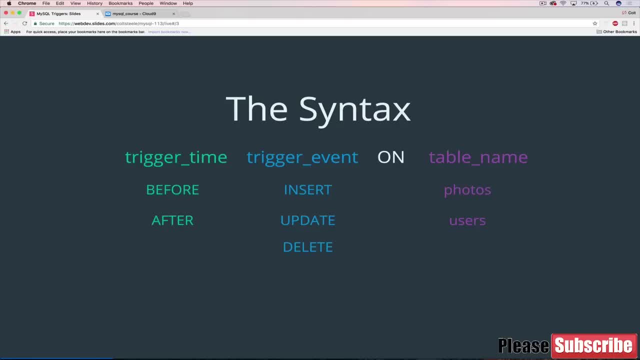 For instance, you don't want to let somebody sign up for your application unless they have an age that's greater than 18.. You can actually write a trigger in MySQL to prevent that creation or that insert from happening if the age is less than 18.. 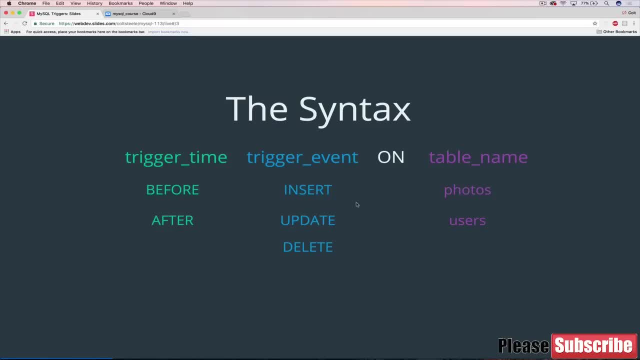 Now the reason I say that it might not be the best use is that you could also do that in your application code. So if you have a web app, an iOS app, a computer app, it's much easier to write code that just says: is this age less than 18?? 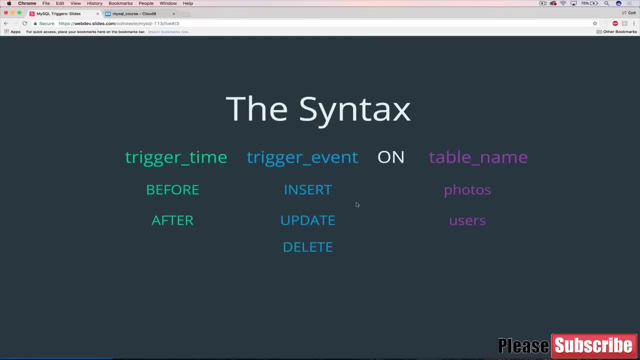 Well then, don't even try to insert it into the database. But because this is a course on MySQL, I am going to show you how to do those validations. In fact, it's going to be the first thing we do, And the way that that works is you run code before inserting into a table. 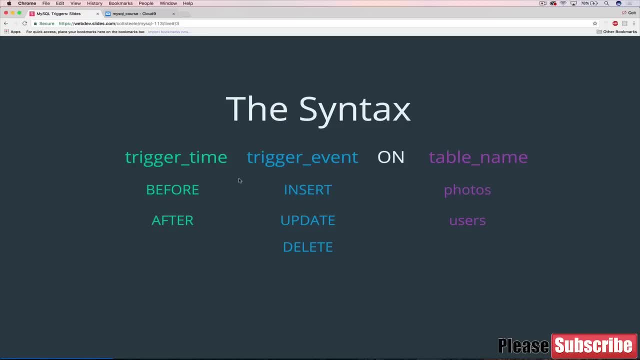 So we would have run this code that checks if age is less than 18 right before inserting into the user's table. So we'll do that. But then the second category has to do with manipulating, creating, deleting other tables. So we would have a table that is relative to your trigger table. 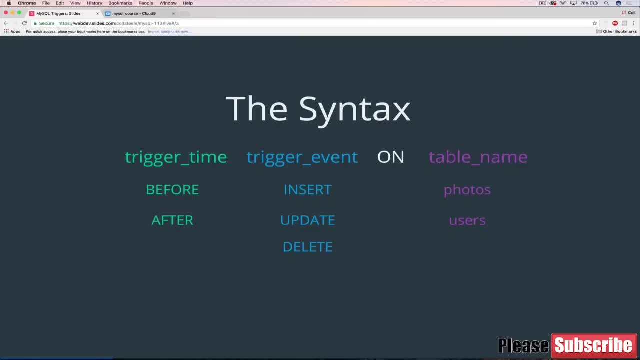 So the example at all I'll give that we're going to do: if we have our Instagram data where you can follow, or any social network really where you can follow people you have friendships, it might be useful to actually know when somebody unfollows. 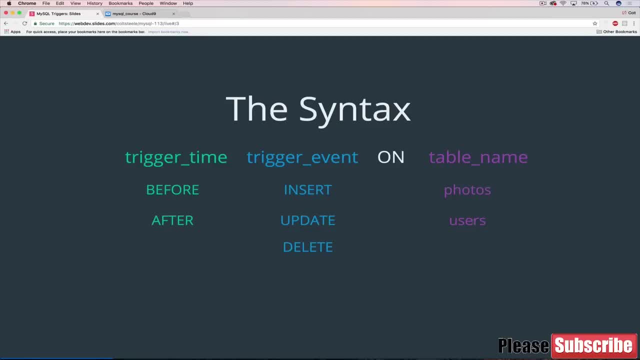 someone. if we're a company, we want that data. It could be relevant, We could. I don't know. we could sell it or it would help us understand when certain ads, ad campaigns- backfired maybe and I started unfollowing, or our users started. 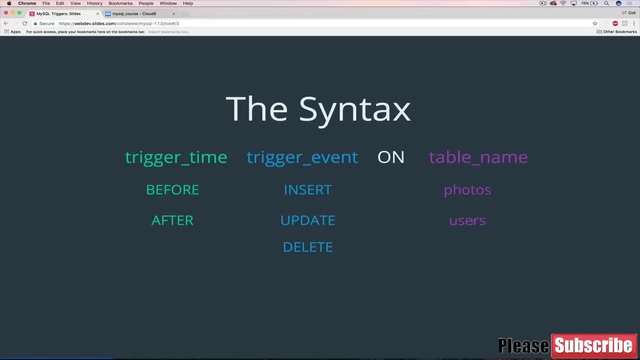 following particular accounts. Well, currently, there's no way of keeping track of that. If a user unfollows someone, if they delete their following relationship, essentially it's gone. What we could do, though, is use a trigger to say OK right after a follow is deleted. 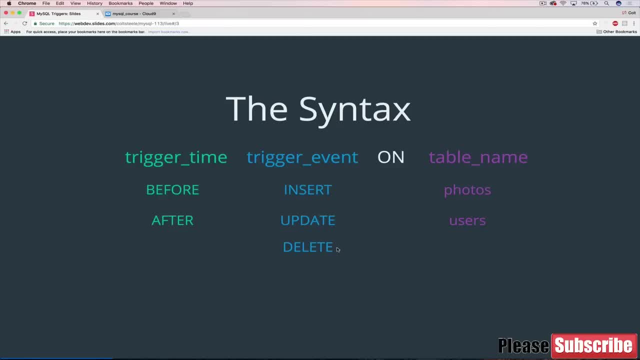 we're going to create some new row, So you can think of it as sort of logging your history, which is a common use for triggers. So that's just one example of two different ways of using triggers. We're actually going to see three. 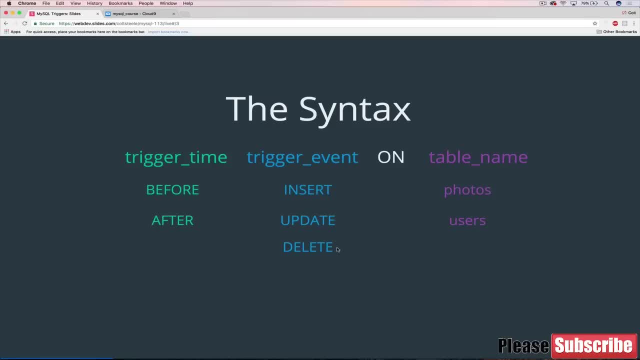 Different examples in this section, but those are the two broad categories. So validating your data, and then the second one is manipulating other tables based off of an initial table triggering that action. So I think it will make a lot more sense once you dive into the code. 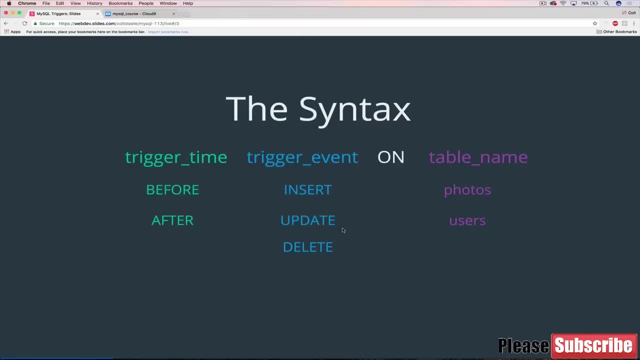 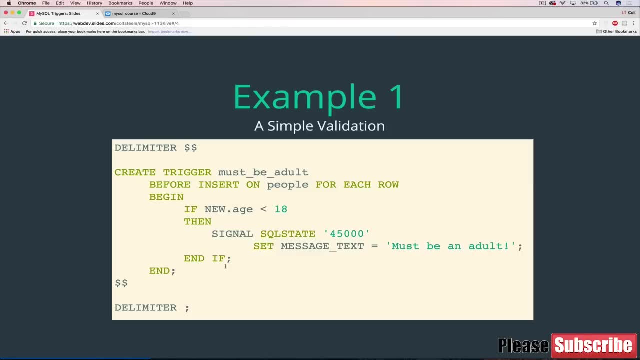 So in the next video we're going to go ahead and create our very first trigger. OK, welcome back. In this video we're going to create our very first trigger And, as a heads up, there's a lot of new code, a lot of syntax. 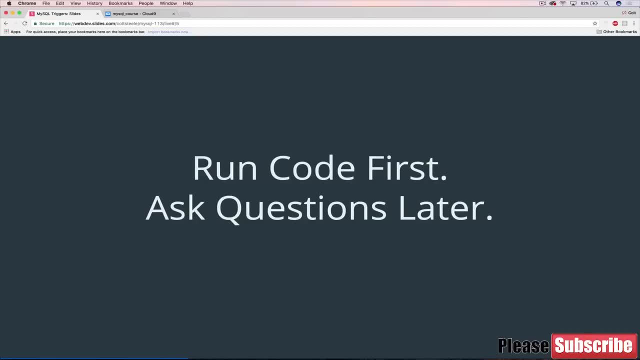 The way that this is going to work is that we're going to run the code first And then we'll ask questions later, which is maybe not always the best approach, But I think here it will help just illustrate how things work- Kind of the overall goal, because you can get lost in the woods. 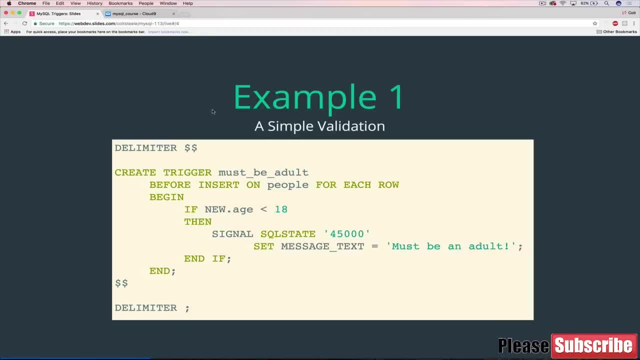 Is that the expression? Whatever? You'll get lost potentially if you focus on these new things like this here, this here, all this stuff here that we've never seen before, And I don't want you to get hung up on that, But we will address it in future videos, the next three videos after this, in fact. 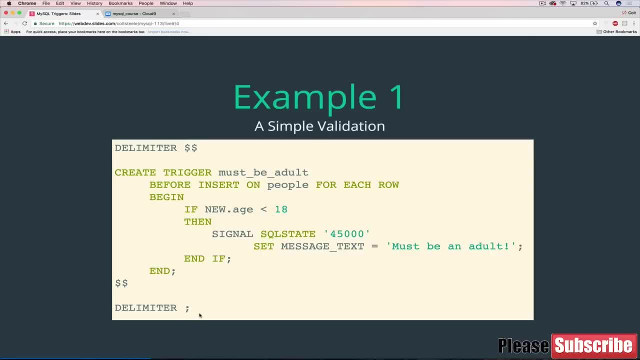 So in this one we're just going to get this running and see that it works And what it is. it's a very simple validation that basically we have a user's table with any data- let's say name and age, username and age- and all that we want to do is prevent. 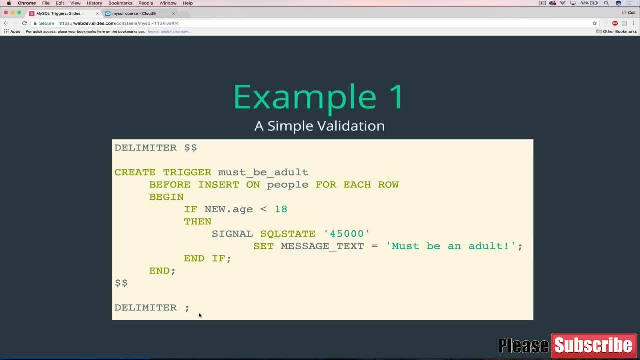 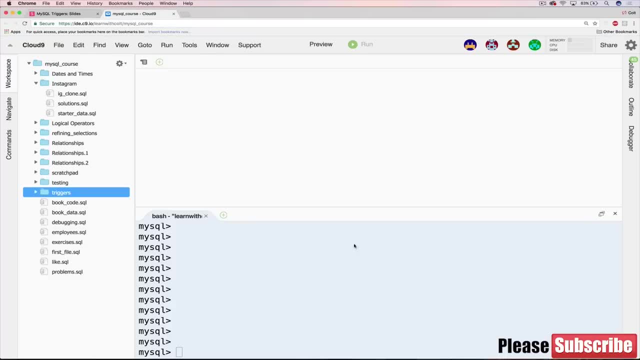 new users from being created if their age is less than 18.. So it's pretty straightforward The idea behind it. like I said in the previous video, it typically would be better to actually do this on the client side If your application, rather than waiting for the insert statement to get to or 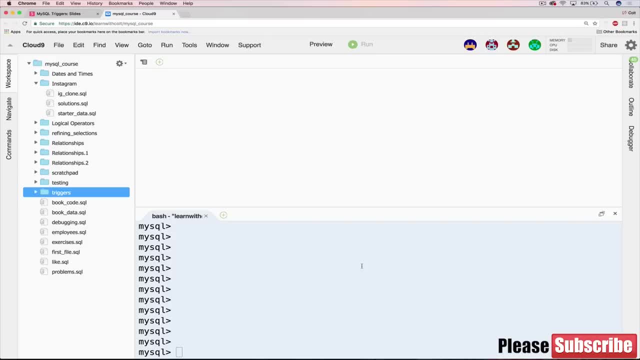 rather than initiating a statement, sending some code to your database, having the database try and insert it and then realizing, hey, this is age, is less than 18, then sending an error back to the client side. That can take time. 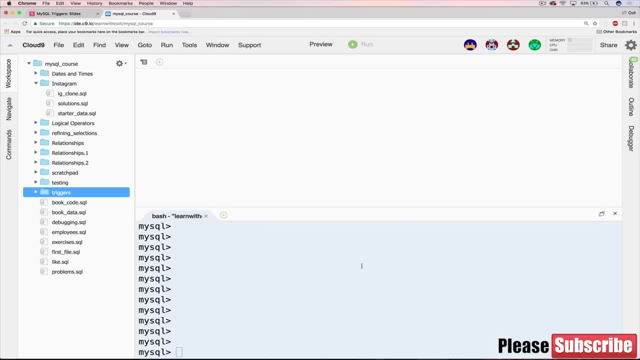 It's much better to just say, on the client side, let's say, of a web app: have a validation on the form that is going to check: is age less than 18 on this form? Well then, don't let the user submit the button, or don't. 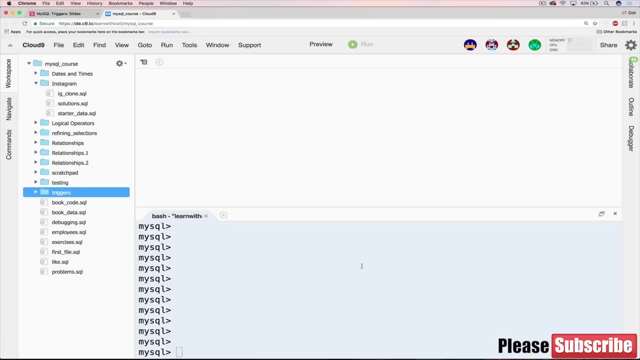 let them click the button or display an error message or something like that, rather than bothering with all this database stuff. But it's important to know that you can do this. I'm going to show it to you And it's a nice simple example. 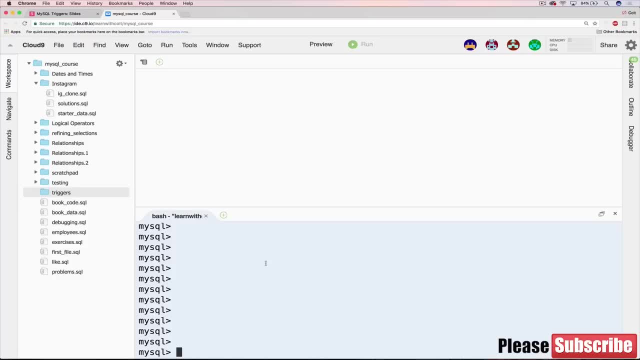 So a couple of things. I'm in a new folder here just called Triggers. I'm going to make a new database as well, And I guess this is a good time- as good a time as any- to let you know that I have seriously injured my wrist on one hand. 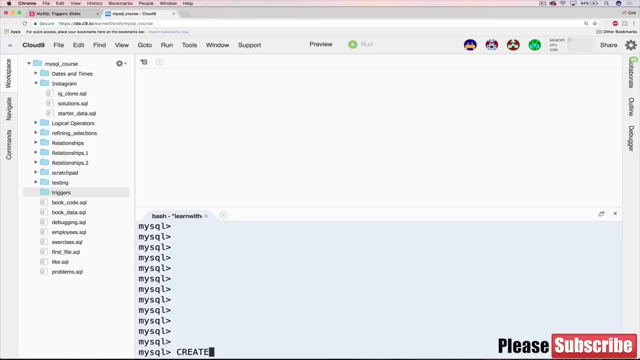 So I'm typing one handed. I'll try and edit around it. Hopefully it's not too noticeable. So we've got create database and I'm just going to call this one Trigger Demo. Oh man, Okay, here we go. Then we're going to use that. 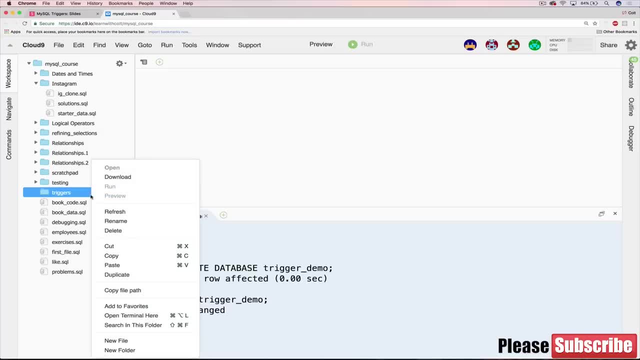 All right, Now I'm going to make a new file just while I'm here, And I'll just call this users dot SQL, And we're going to make a simple table, create table. very, very simple users And, like I said, it's only going to have- let's go with- username. 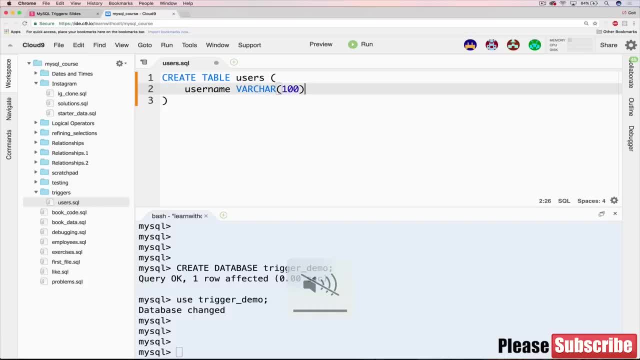 which will be a Varchar, and then we'll also have age, which is an int, And that's it Okay, so we can go ahead and run that, just to validate, to check that it works. So we'll do. source users dot SQL. 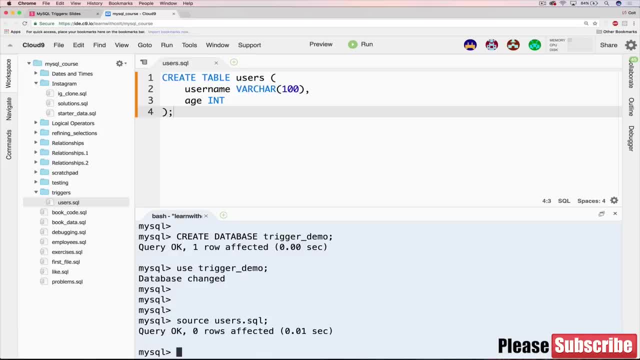 I ran this in the same directory, Okay. Okay, We should be able to do show tables and I should be able to insert a user. Let's do insert into users and we'll do. username age Should all be boring review at this point. 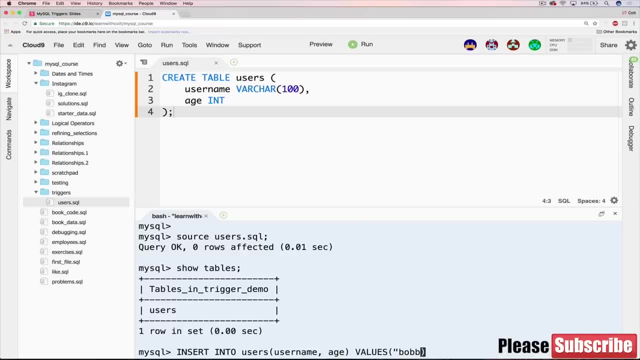 We'll go with Bobby and ages. Let's go with 22,, 23.. Okay, there we go, And as always, we select star from users, just verifying that everything works, All right. Pretty boring stuff. Now we're going to go ahead and create this trigger. 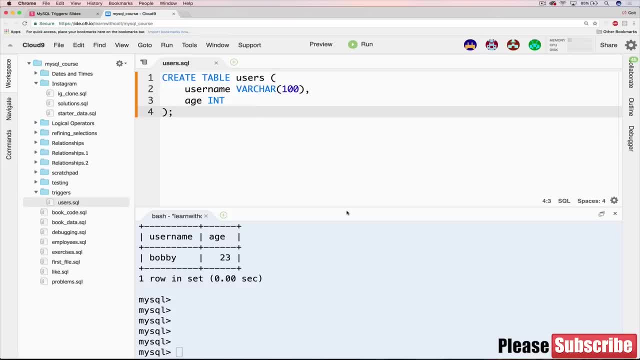 And what this trigger is going to do is, right before a piece of data is inserted into users, right before a new row is created, we're going to say: hang on, hang on, There's a trigger that's just been triggered And it's going to check if this new user row, if the age is less than 18.. 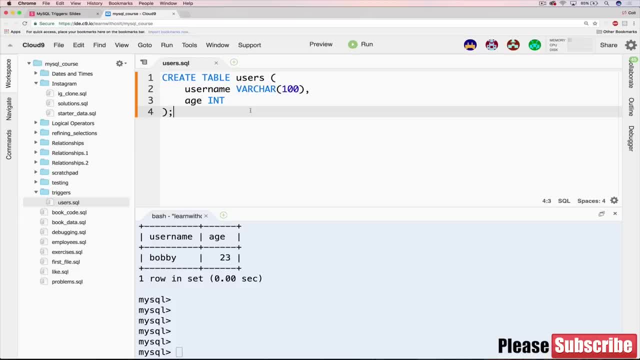 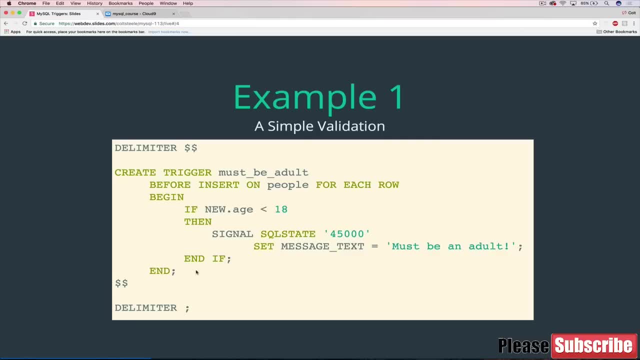 And if it is, then we're going to throw an error. We're not going to let it happen. Otherwise, proceed normally and insert the user. So the syntax: I've already typed it up here. You can just copy this if you'd like. 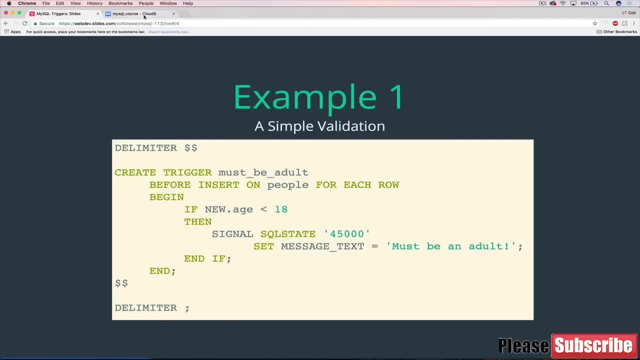 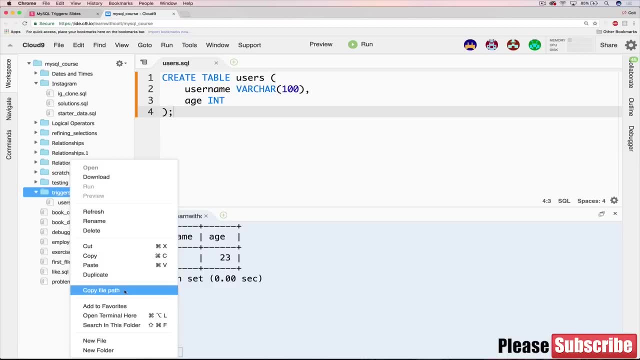 It's going to be easier. Like I said, we'll go over the ins and outs of it as we go through this section, But to start we'll just copy it And what I'll do is make a new file. You don't have to. 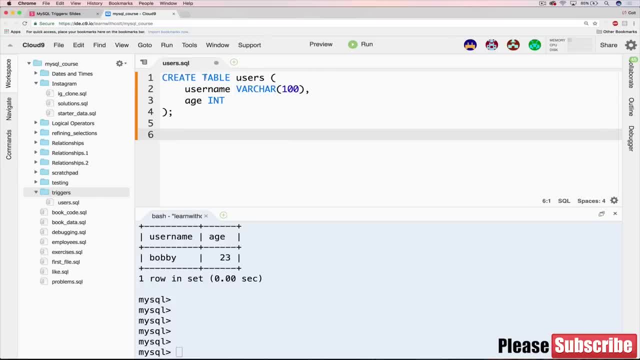 You could just add it down here and just rerun this whole file, But then you've already created the users table, And so you would have to recreate it and drop it and then recreate it. Anyway, it doesn't really matter, I'm going to make a separate file. 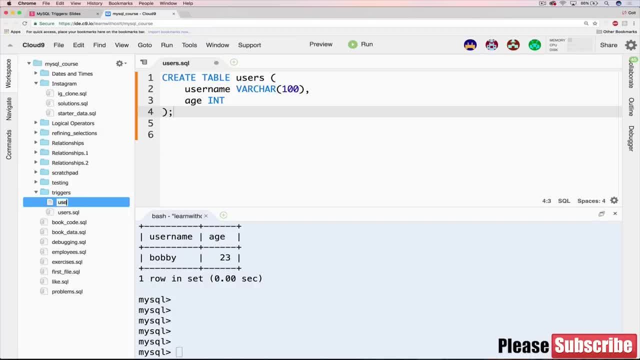 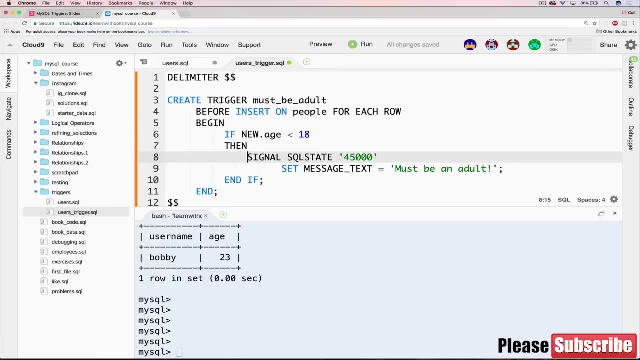 I think it's good to keep your triggers separate, So I'm just going to call this users trigger dot SQL. OK, and then I'm just going to paste it in and hit save, And then I'm just going to source this file just like any other SQL file that we've run. 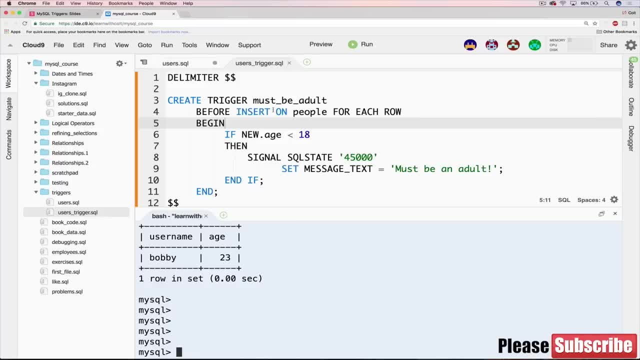 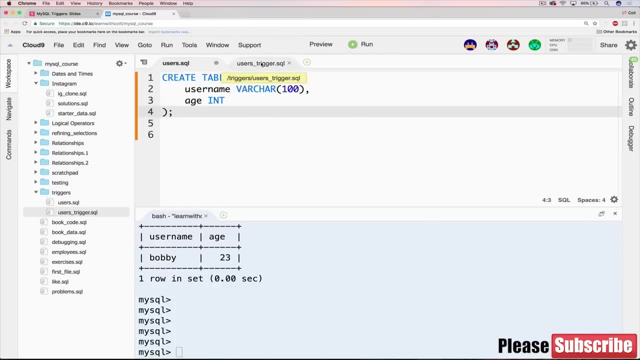 It's just a little different than what we've done before. This is sort of like meta SQL, where we're not actually interacting with the database immediately, we're not creating tables, we're not inserting things, We're creating restrictions or triggers on another table. 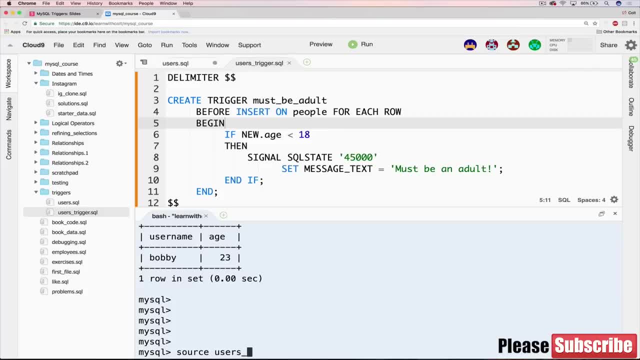 OK, so I'm going to source it. I called it users trigger dot SQL. Oh, actually, before that, let me just verify that you can create a user who is less than 18.. So let's say Sally is 16.. 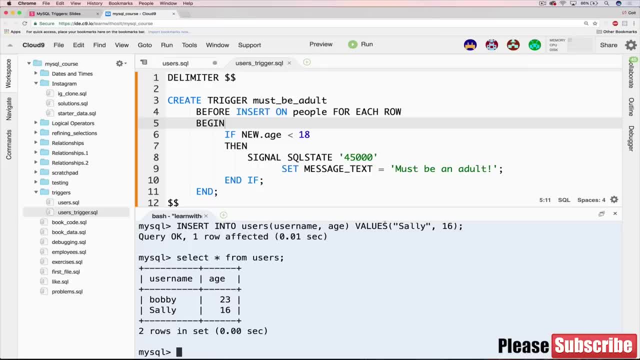 And that works just fine. They're both in there. But now when we source our users, underscore trigger dot SQL- we get this silly error, which is my fault, And rather than editing around this, I'm actually going to leave it. It's somewhat educational. 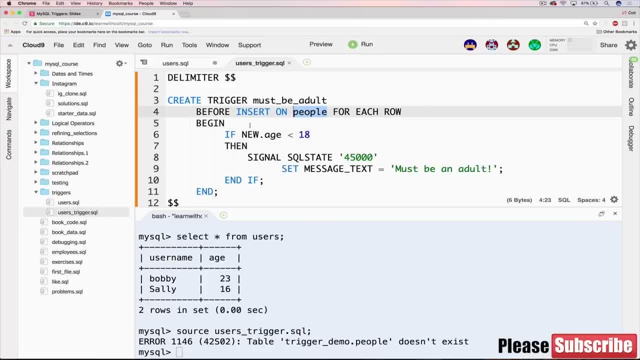 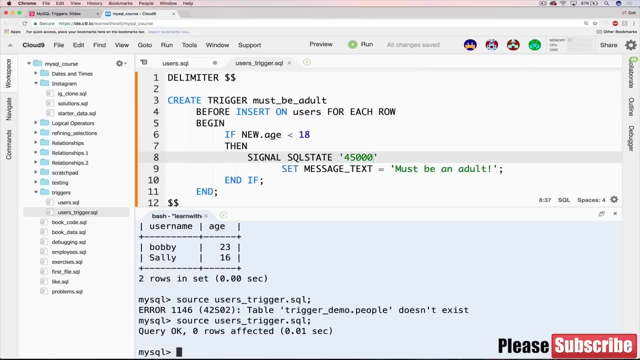 I have a table called people that it's expecting before insert on people. Well, there is no people table in this database, It is a users table, So let's recreate that. OK, so now I do that And we get this message that, like we get every other time, something works. query. 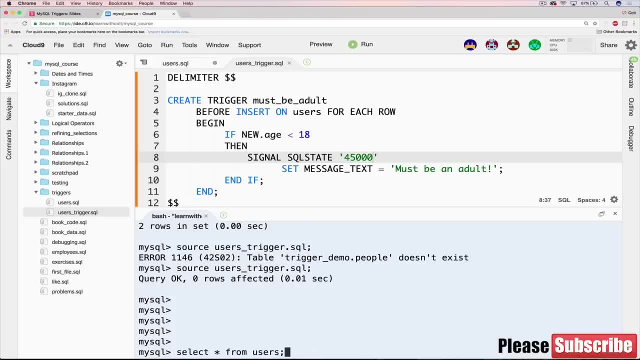 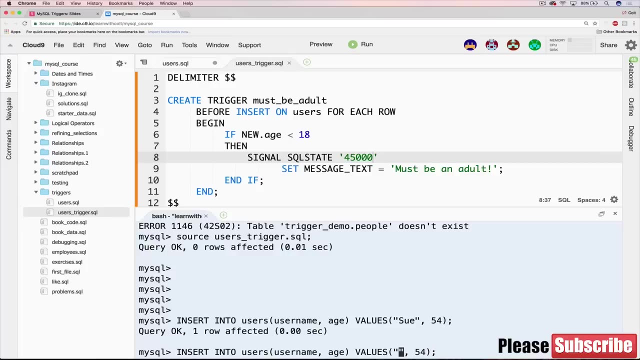 OK, now let's see what happens. So let's start off with something we know works, Like: let's do Sue, who is 54. That should work and it does work. But now let's do man. this is the hardest part. 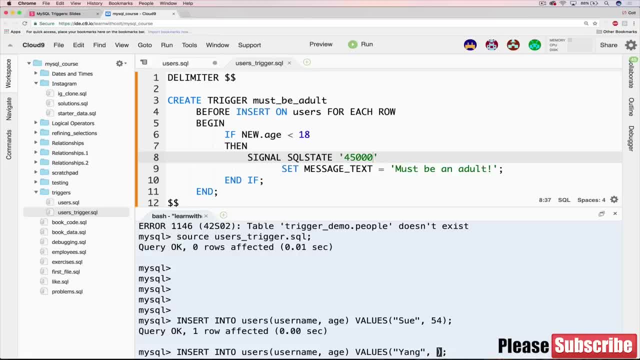 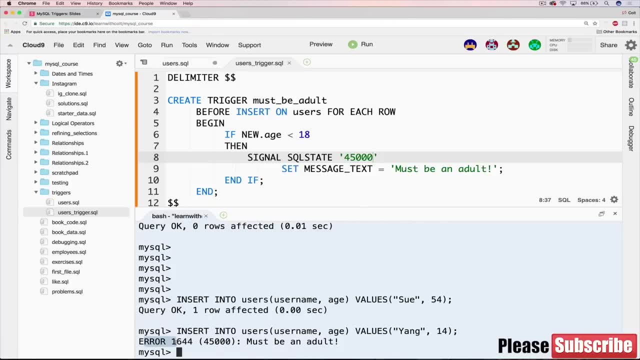 Let's go with Yang, Who is Fourteen less than 18. And we get our message error. We'll talk about this: 16,, 44,, 45,000,. all that fun stuff must be an adult, And it's not just an error. 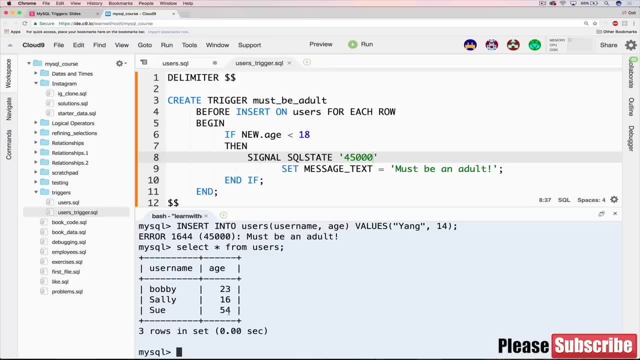 If we actually go select all our users, Yang doesn't get inserted. So it's not just like an error that gets thrown out just as a FYI, but it also prevents things from from actually being inserted. So that's the basics. We've got it working. 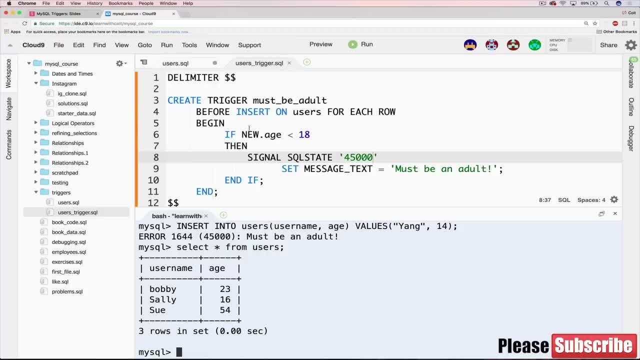 In the next video I'm going to break down some of the new pieces of code, in particular: what the heck this is here and here and here Also, what this new thing is, new age And, most importantly, what is signal sequel state. 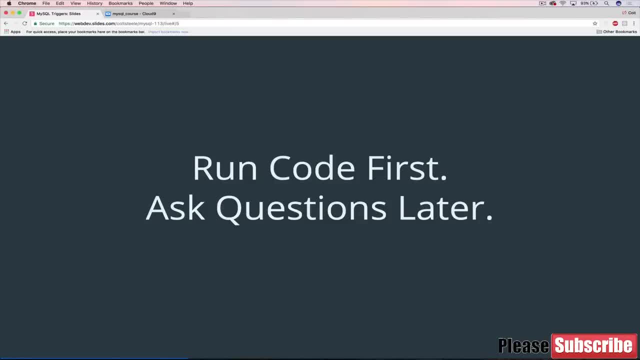 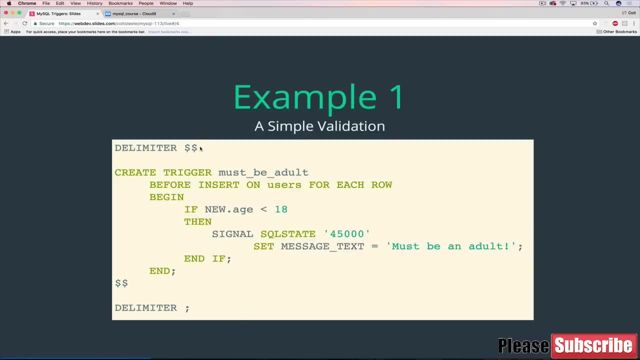 Forty five thousand message text, all this stuff, All right. So we ran the code first. Now we're asking the questions. So, going back to the code here, there's a couple of things I want to point out. We'll come back to the delimiter stuff, the beginning and end. 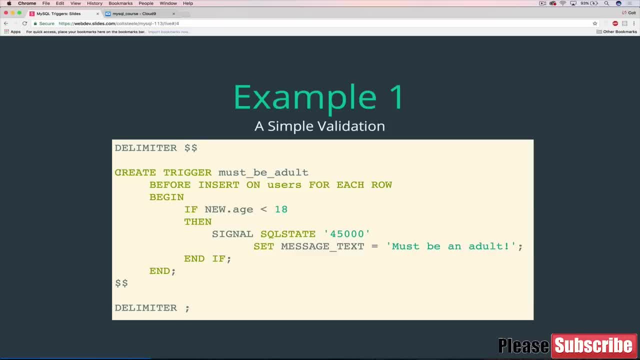 But I want to focus first on the basic syntax. So create trigger that standard, Give it a name. I called it must be adult. You can call it whatever you want. It doesn't actually have any impact. Again, it's really a label, so that if you do want to delete this trigger later on, 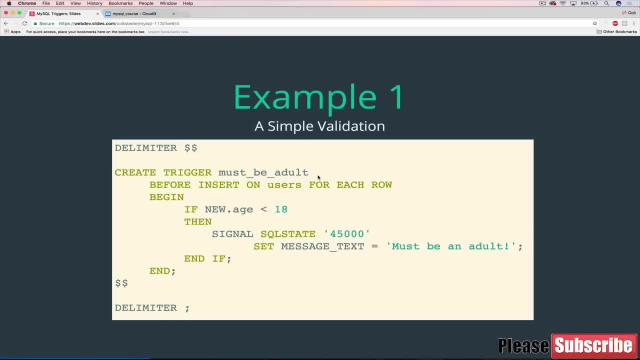 you have a name to call it by so that we can delete. must be adult, But give it something meaningful. Then we have the important stuff. So this is the meat of the trigger. We have our trigger time, the trigger event and the trigger table. 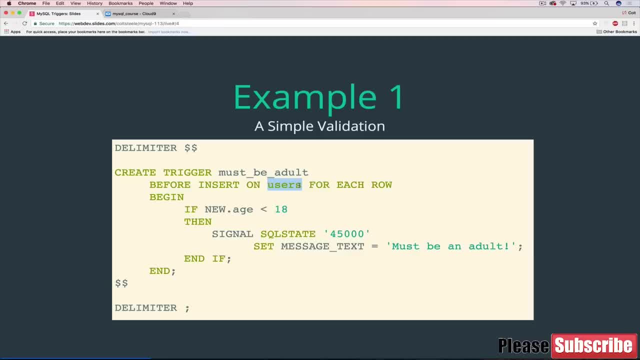 So this is the user's table. That's the simplest one to start with. We want to run this code here right before something is inserted into the user's table. Now, if we had said after, it wouldn't really do much because it wouldn't. 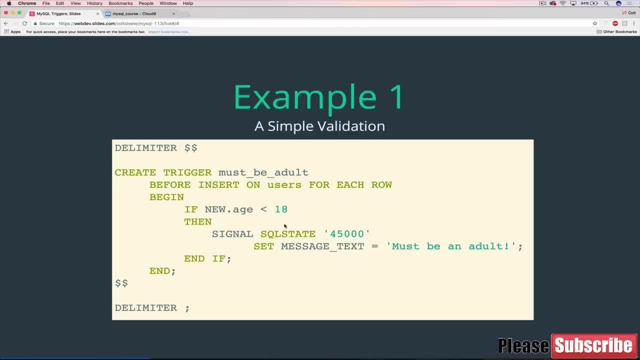 prevent a user from being inserted if their age is under 18.. It would still check and it would still give you an error if age was less less than 18. But it still would insert it because it would be running afterwards. So it's not really a validator. 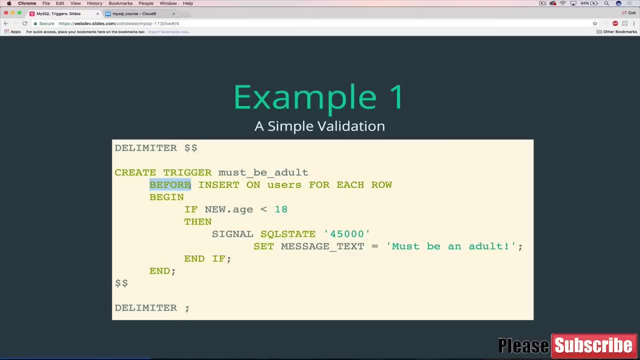 So because of that we definitely want to have before, But I will be showing you where you can use after in another example just a couple of videos, But in this case before insert, So it will run immediately before anything is inserted into the user's table. 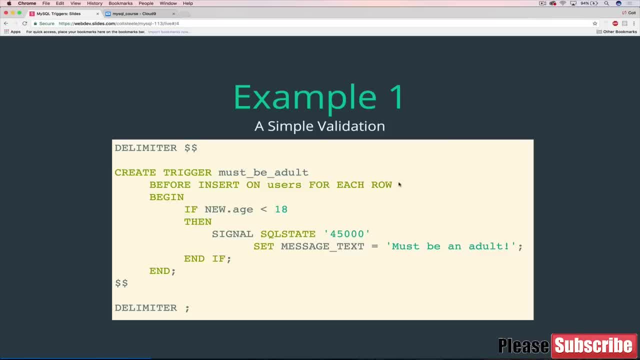 Then we have for each row. that's just default syntax. Begin and end. Notice a semicolon here. we'll come back to that, And whatever is in between begin and end is the actual code. This is SQL code that runs every time right before something is inserted into users. 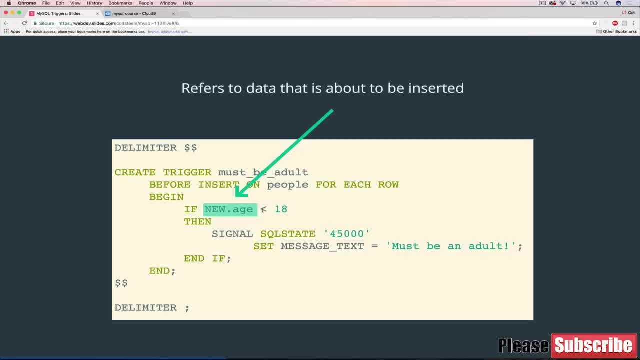 So let's start off by talking about this: if new dot age less than 18.. So, first of all, we have this if syntax, where you have if then and then end if, which you've seen before. But, more importantly, we have new dot age, and new in this case is just a placeholder. 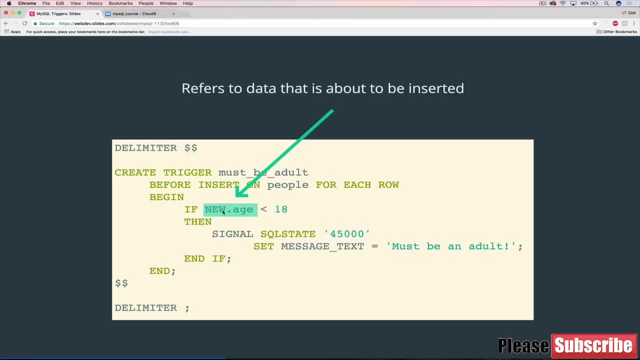 It's referring to the data that is attempting to be inserted. It's referring to the new user that's going to be inserted into the table. So if new dot age is less than 18, do this. Otherwise don't do anything. 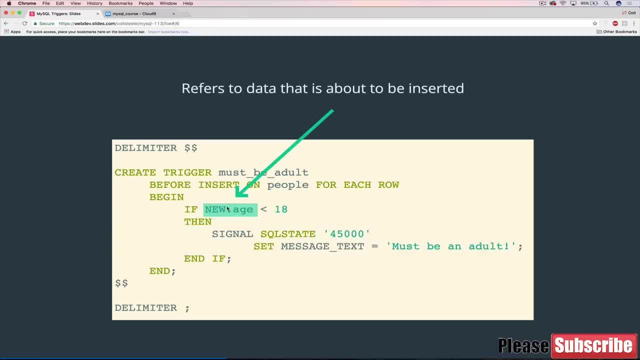 There's also an old old that goes along with new that we'll see later on. Once we've deleted something, we want to have access to the data that was deleted. We can use old dot, whatever. So new age less than 18.. 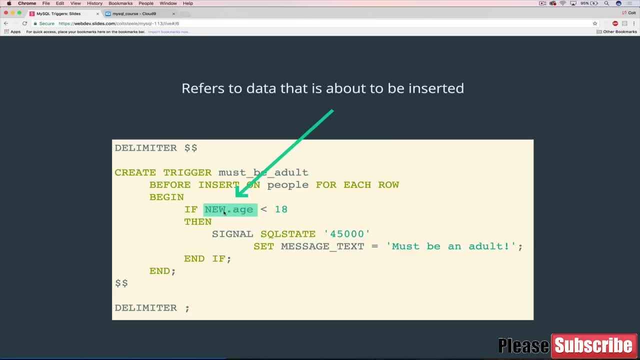 New is a placeholder for whatever user is being inserted. Then we move on to slightly trickier thing. What the heck is this signal SQL state 45,000. set message text: equals must be an adult, So the second part is probably more self-explanatory. 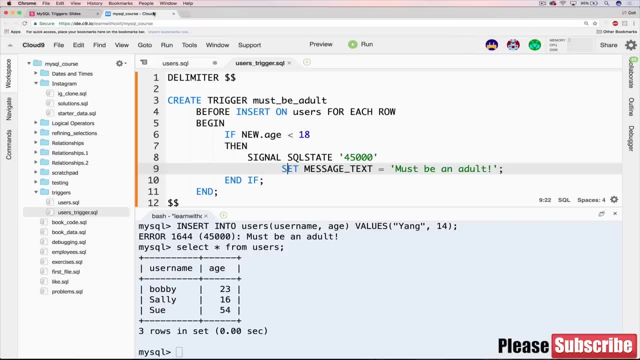 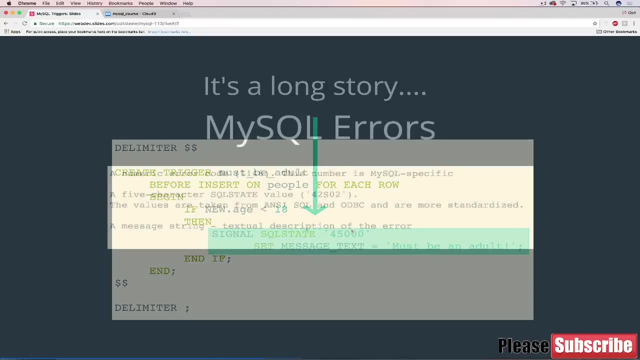 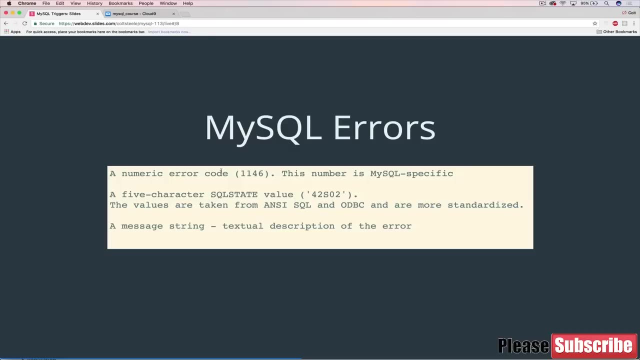 Set message text must be an adult. We saw that message text here: must be an adult. But the SQL state thing is kind of confusing. So according to the MySQL docs, there are three components to a MySQL error. There's a numeric error code. 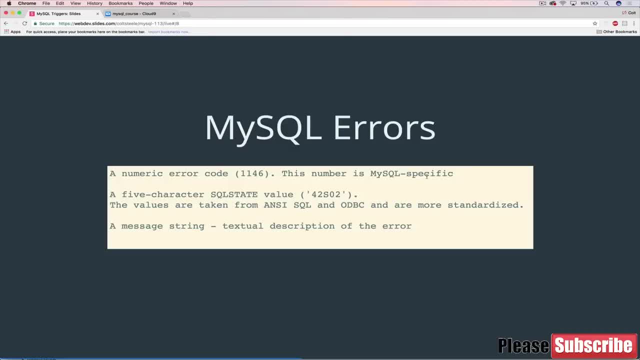 1146 is a common one, And these are actually MySQL specific error codes. But then there's these other things called SQL states, And that's what we care more about in this situation. It's a five character value, It's not just numeric. 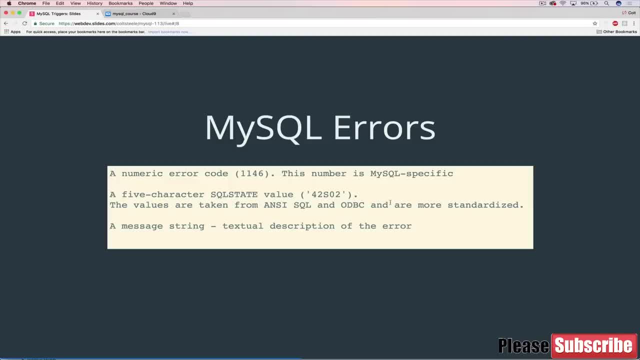 It can have letters and they're taking blah, blah, blah, blah blah. This is from the docs, by the way, if you want to read more about it. But they're more standardized across SQL databases, So it's not just MySQL specific. 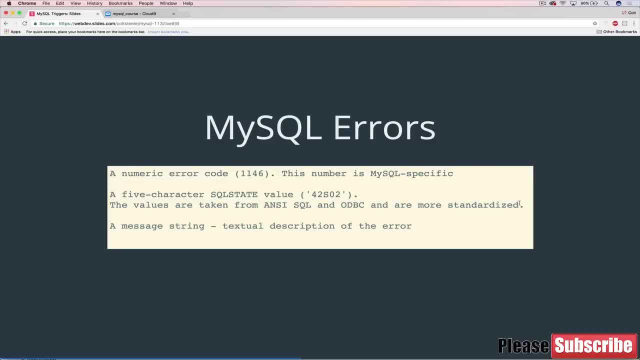 This signal state code is recognized essentially across different databases, And then along with that there's always a message string, a textual description of the error. So that's important for humans: for us to recognize what's happening, But for our code to recognize what's going on, it's much easier to work. 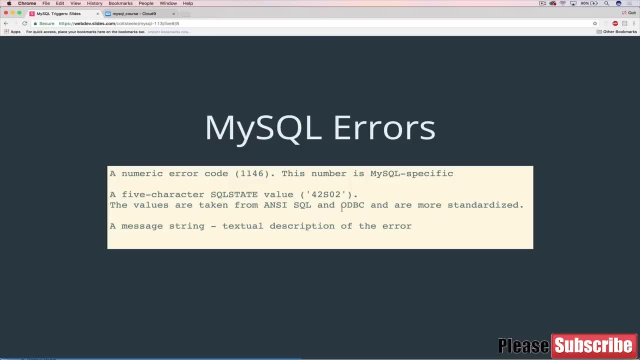 with these numeric values or these SQL state values. Those are easier to recognize. You can write code that says, hey, if we get an error equal to 42SO2, then do this, Rather than saying if we get an error that says exactly must be a number must be greater than 18.. 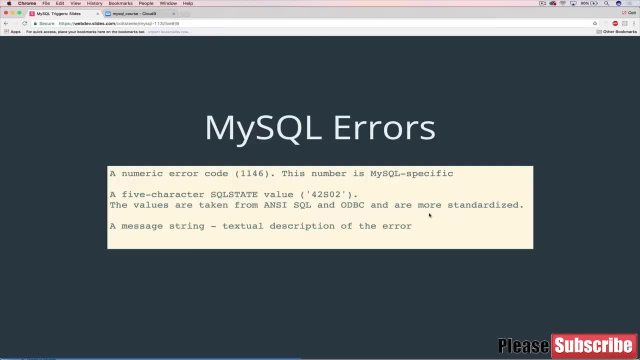 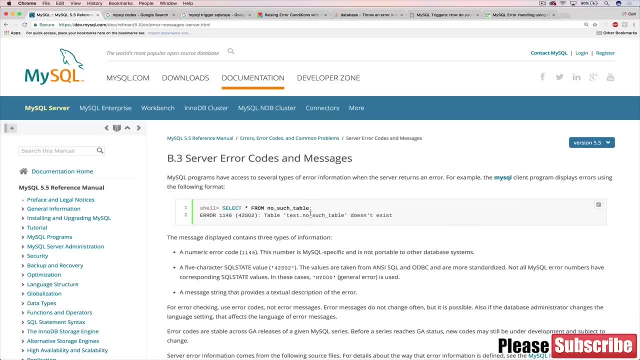 There's sort of a lot of wiggle room there, depending on how it is implemented. But these numbers, these hard coded values that never change, are much easier to check against. And as a side note on the MySQL docs, there's this page: server error codes. 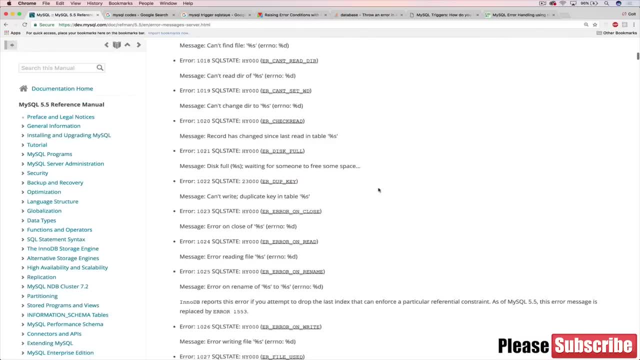 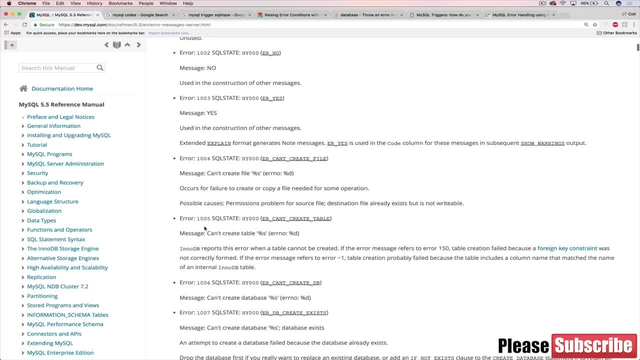 and messages. If you scroll down you'll see there are tons of these messages and there's these errors and accompanying messages. Let's just pick one. Let's say here's one here Error. So the MySQL error code is 1005.. 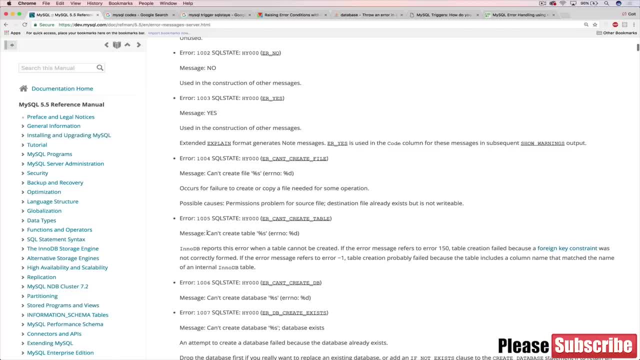 The SQL state is HY000. And the message is: can't create table, And then inside of here it will put the name of the table you try and create. So this would happen if you tried to create a table for some reason that you. 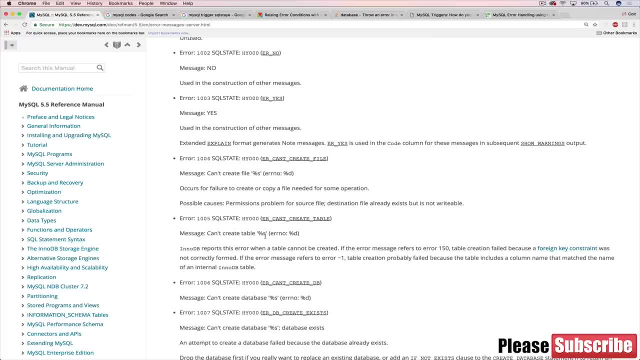 couldn't, whether I'm trying to think of actually how exactly this would happen. It says a foreign key constraint Potentially there's. well, it doesn't matter that much. However, you get this error, It will show you the error code, the SQL state code and the message. 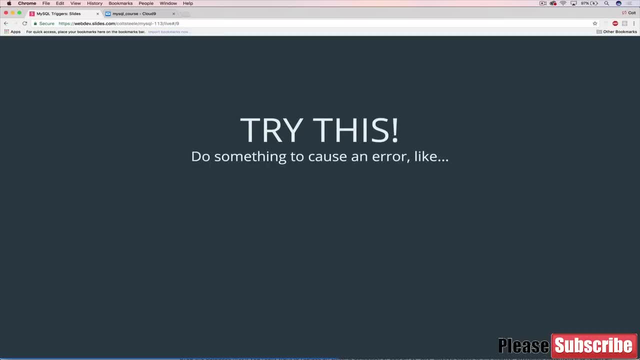 And in fact, if we go, try this, cause an error on your own. Feel free to do whatever you want to cause an error, But here's one we could do: Select star from this table that we know doesn't exist, Just gibberish. 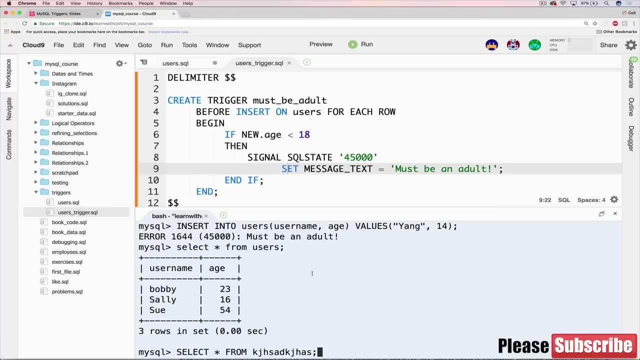 If we try and do that, go over here- We get an error. so it says error and then we have 1146.. So that error code Is the MySQL specific code. Then we have the SQL state for two: S02.. And then we have this text: table trigger: demo dot. blah, blah, blah, blah, blah. 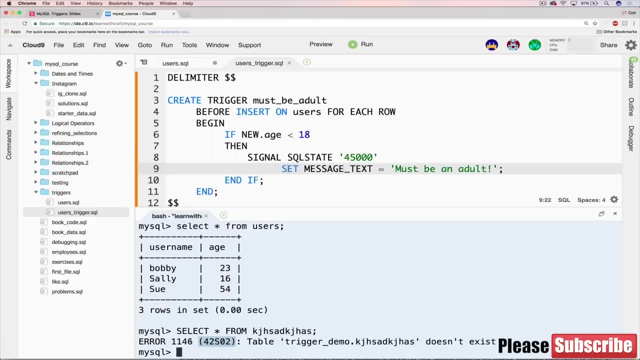 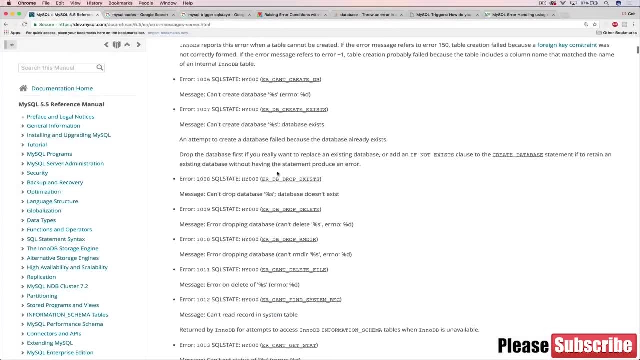 Doesn't exist. So this is the message, This is a SQL state and this is the code. What we care about is the SQL state and then the message, And if we go over to the docs again and we try and find that code, 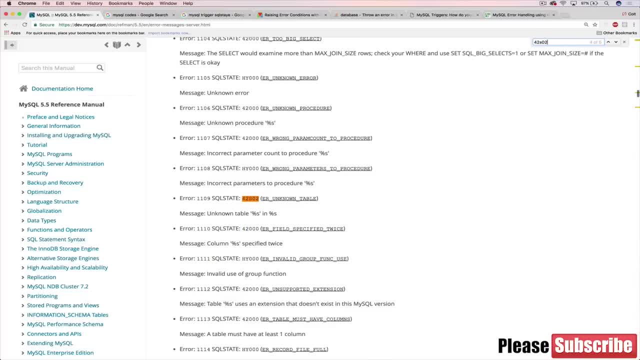 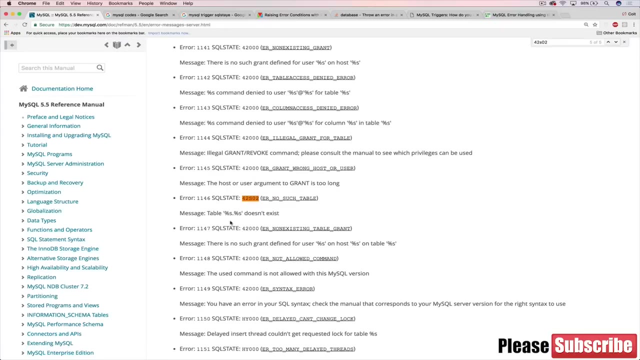 So we had. the SQL state was for two S02.. You can see that it shows up a couple of times. There's an unknown table message: unknown table, but there's also bad table. And is there another one? Yes, Table doesn't exist. 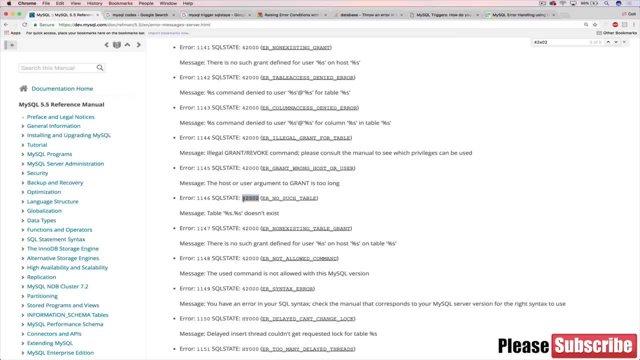 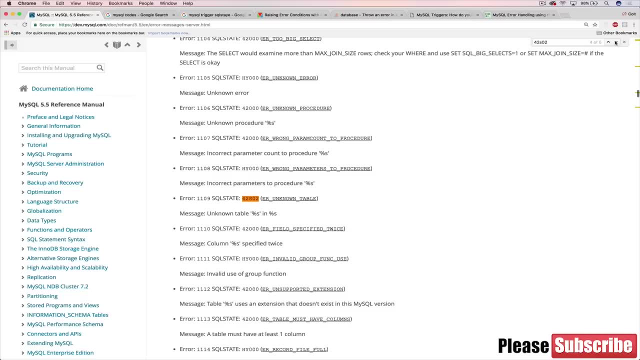 Error: No such table. So those all use the same SQL state but they use a different MySQL error. There we go, So 1051 versus 1109.. This is really getting into stuff that doesn't matter that much to us. 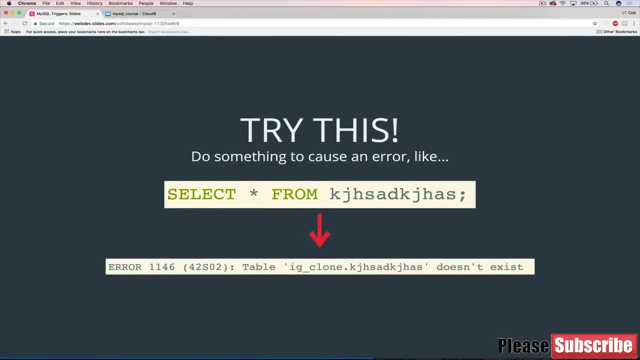 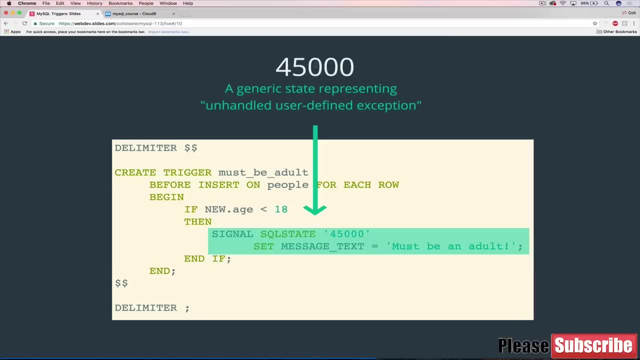 And the reason that it doesn't matter to us is that we're going to use one and only one SQL state, which is 45,000.. So 45,000 is sort of like a wild card state, that is generic and it represents an unhandled user defined exception. 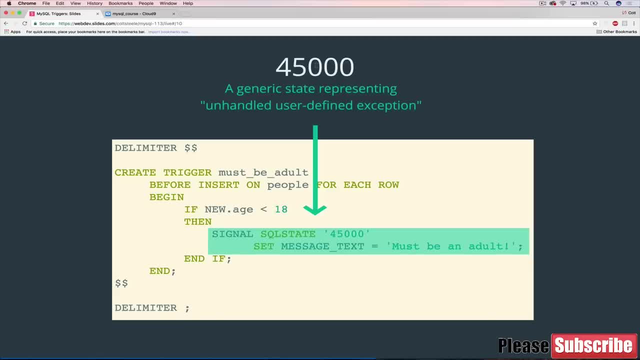 So it's kind of just left out there for us to use it for developers to return 45,000 as a way of saying, hey, this is something I've come up with. This is not a MySQL. This is not a SQL thing, like you know. 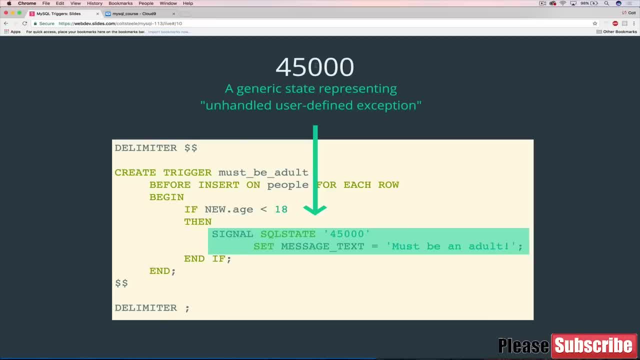 an unknown table or a syntax error or something. This is something that I've defined and I've set the message. So signal SQL state in quotes 45,000 is what we'll have any time we want to throw an error. then we have set message text and then that's important. 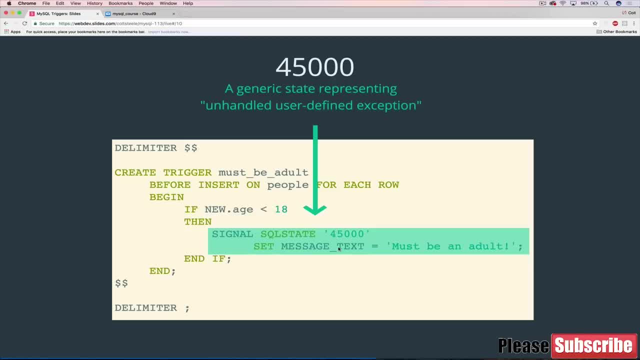 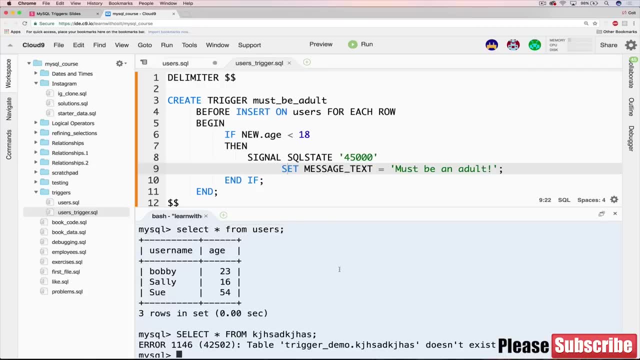 That has to be set message text. It can't be set anything else. Set message text equal to whatever message we want returned alongside that. And then if we go look at what happens, just to refresh your memory up here when we try that, we get error. 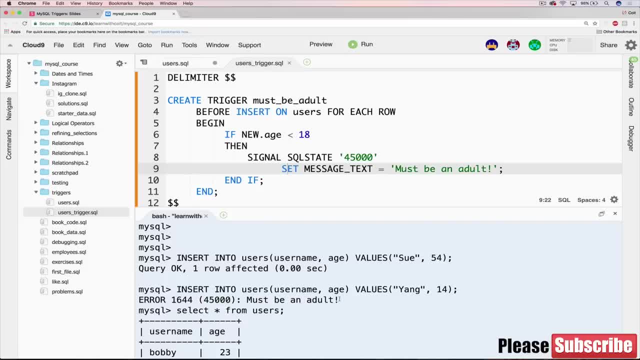 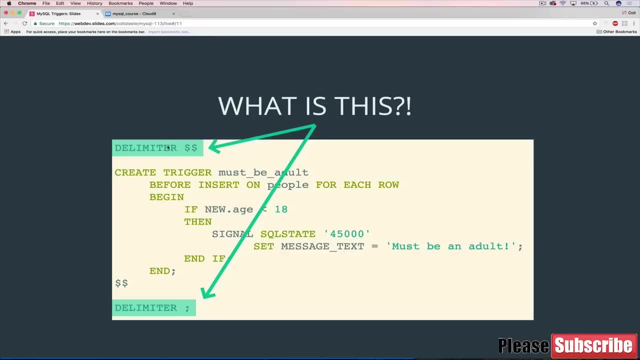 Here's our SQL state. and then must be an adult. So that's the basics of this kind of new stuff in here. But then we move on to what the heck is going on here with this delimiter dollar sign, dollar sign and then two dollar signs here and then delimiter semicolon. 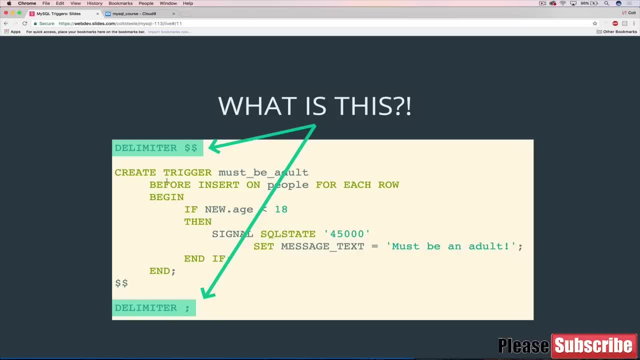 What is that? So, basically, if we take a look at- let me go to a cleaner version of this Back here- if we take a look at the code, we have semicolons in certain places. That's because these are multiple line statements. 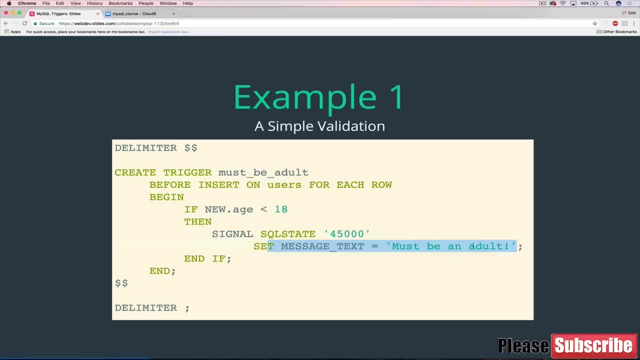 So we need a semicolon after something like setting message text or an if statement or this begin and end. And if we just use a semicolon and didn't have this delimiter, so just pretend this isn't here, All of this, each of these lines, would be treated basically as the end of our code. 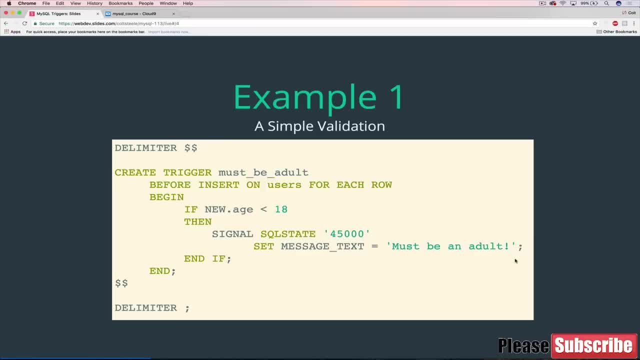 Remember that when my SQL sees a semicolon, by default that is the delimiter And that basically means this is a signal that I'm done with this line. Go ahead and execute it. But we don't want that to happen, So we don't want this thing to be read in and it gets this first semicolon. 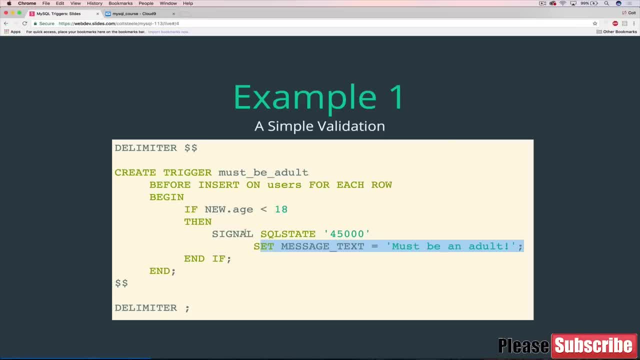 And it says: all right time to execute this. This is the end, because it's not in fact So. what we do instead is change the delimiter temporarily to. it doesn't have to be two dollar signs. I've seen people do it with slashes. 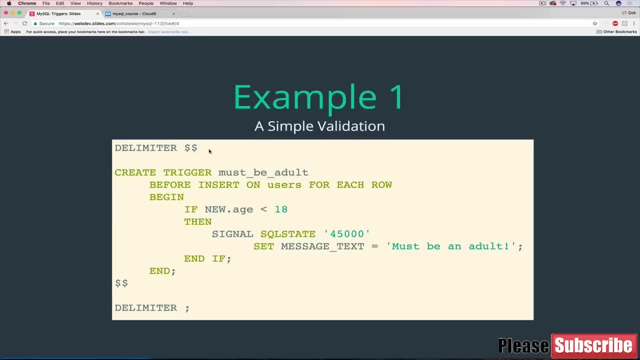 Two dollar signs is most common, though just because it's not used anywhere else. So delimiter space: dollar sign, dollar sign that says OK. from here on out the actual delimiter is two dollar signs. So the end of our code is when you see two dollar signs. 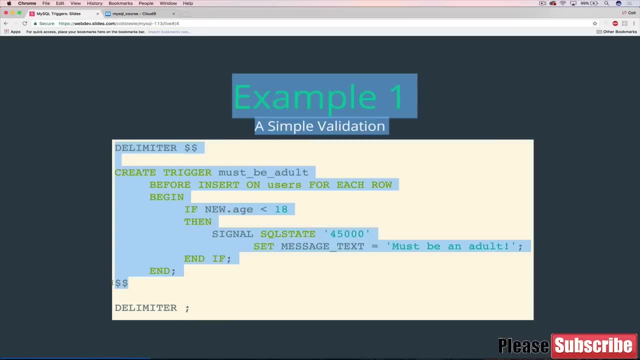 So then all of this is treated as one chunk. We hit the two dollar signs, that says this is the end, and then we can change it back to a semicolon If you didn't have this line- which I've done before accidentally, so we can actually do this now in the console- 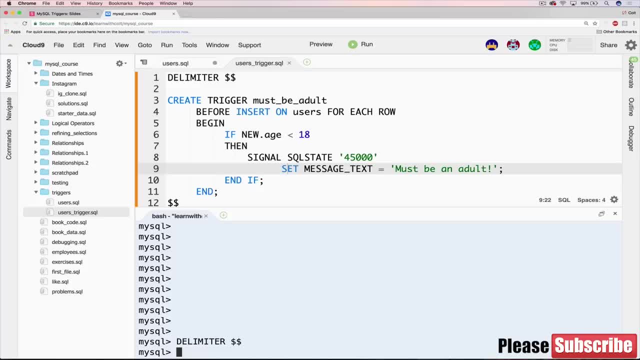 You can just change the delimiter any time you want. So if I run it now and I try and do, let's say, select star from users semicolon and I hit enter, nothing happens. And that's because it thinks that I'm still going. 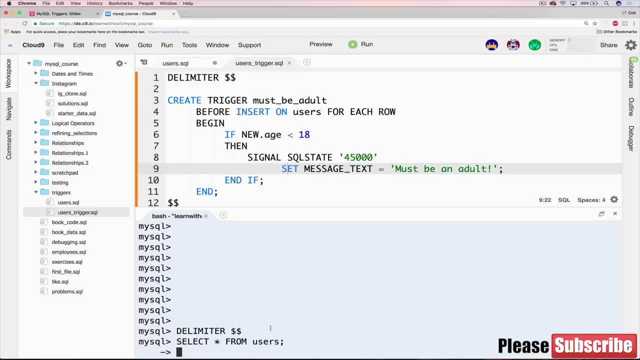 I haven't, it hasn't hit the delimiter. So I add two dollar signs which now says we've hit the end. So you have to use dollar signs now, which can be kind of annoying if you forget. So you can see that now replaces the semicolon. 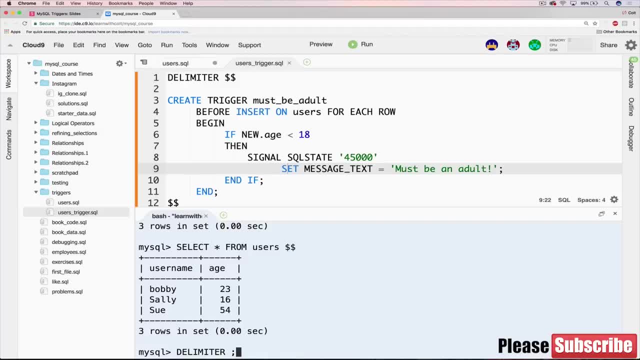 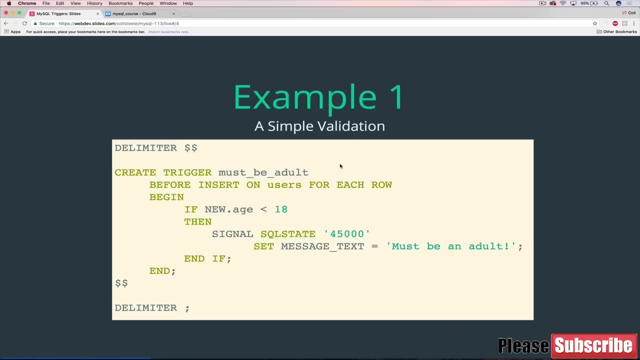 However, we don't really want that, So I'm going to go back and just change it to semicolon, And now semicolon works. So that's all you need to know about the basics here. There's kind of a lot of pieces, but the most important thing- 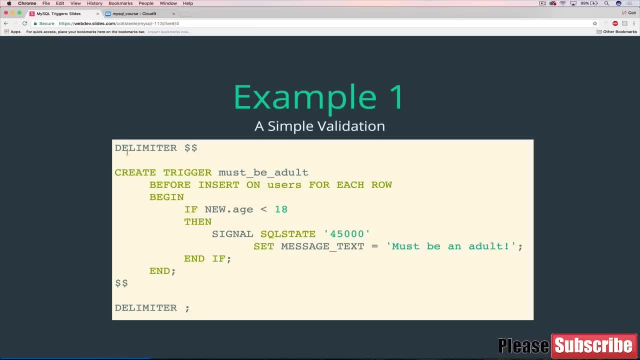 the template for any sort of trigger that you do usually has delimiter up top And then you're using the dollar signs or whatever you set down here And then you have create trigger and a time. then you have a time before or after an action or an event. 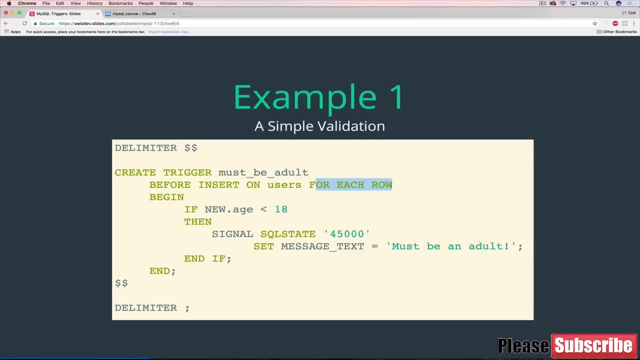 insert, update or delete, and then you have a table and then for each row, begin and end- those always are the same- And then you have something happening inside of there And, just to summarize, new refers to the new piece of data. 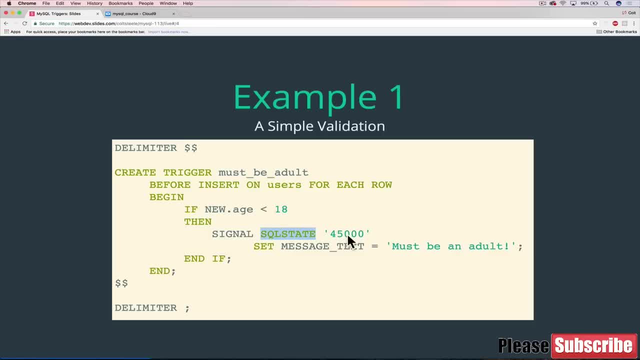 the new row we're trying to insert and then SQL state signal. All that stuff is just involved in sending an error message back. It's kind of a lot, But going forward. we have two more examples. We're not going to spend a lot. 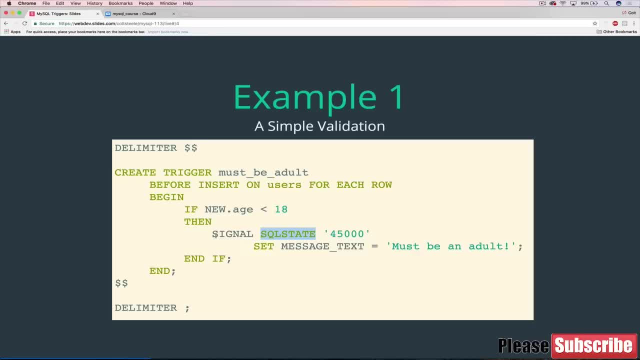 of time on the nitty gritty details. We're just going to get going and just see how they work because, honestly, whenever I create a trigger, I just go up to an old one that I've done before, I copy it and then I tweak it. 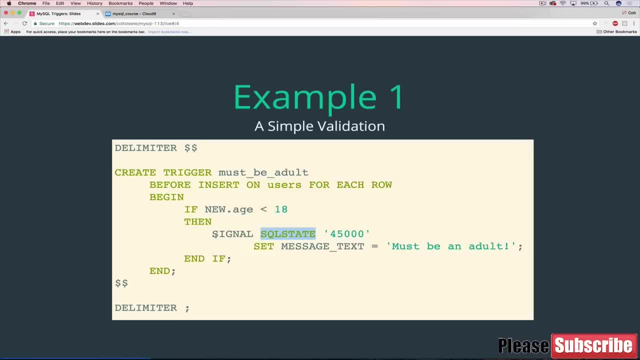 I don't start from scratch like I would with creating a table. You just don't do it that often, So no pressure to feel like you have to memorize all this or take it all to heart immediately, Just kind of be comfortable with understanding it. 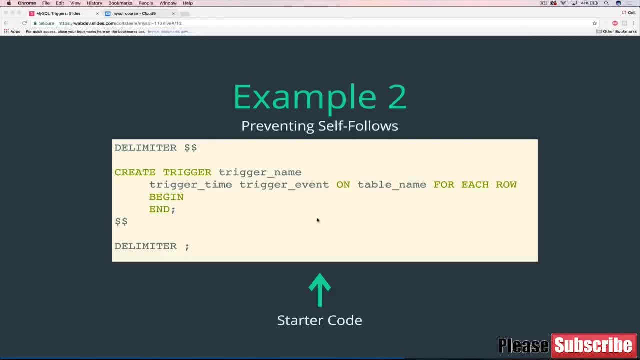 If you see code in front of you, All right. All right, Welcome back. So we're continuing on with triggers. We're going to take a look at another potential trigger we could write And in this case we're going back to the Instagram data. 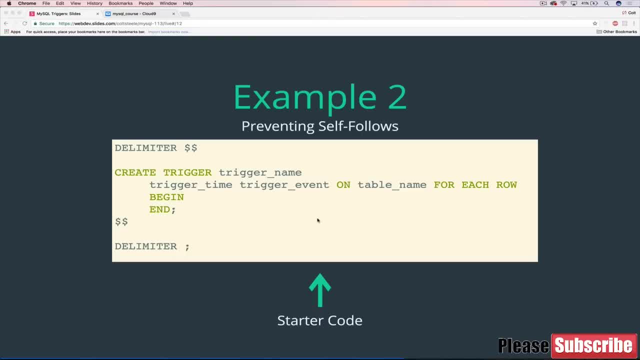 which hopefully is fresh for you. It was just the last section. It's been a couple of weeks for me so I had to refresh my memory on how the data looked. But basically we're going to focus on one table, which is the follows table. 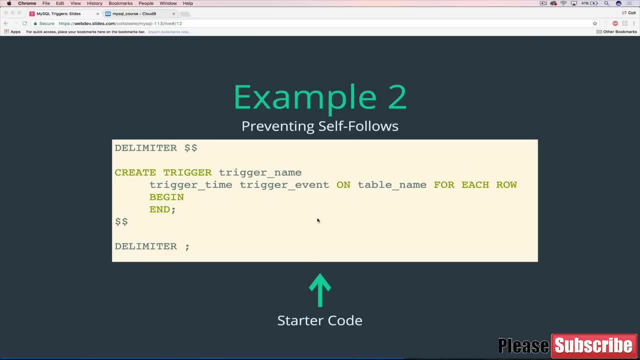 So, remember, we have users and they can follow each other. It's a one way relationship, unlike something like Facebook. It's like Instagram or Twitter, where I can follow someone and it doesn't matter if they follow me back. So So, right now, all that we're storing is: 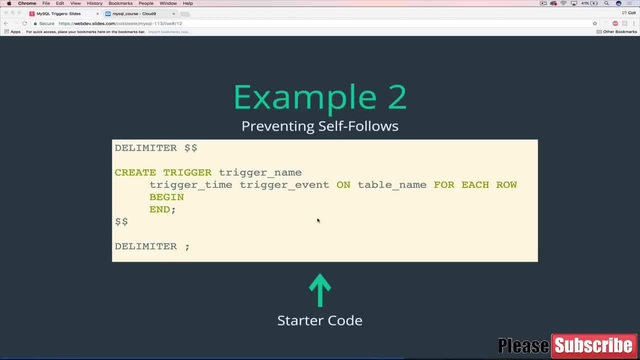 a follower ID and a follow ID and created at potentially, But really it's those two IDs that are important, both foreign keys. What we want to do is prevent users from following themselves, which is something a lot of people have commented on. 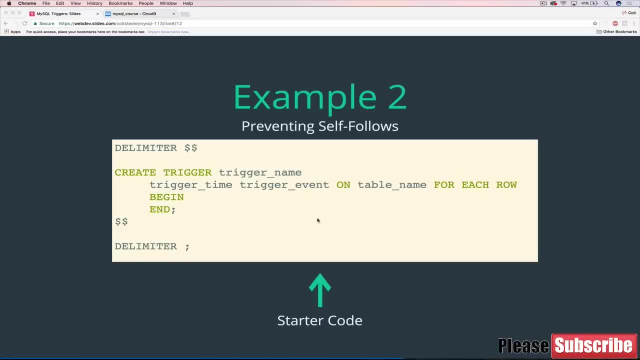 It's a pretty, I mean, it's a. it's a logical thing to want to know about, because it seems like a pretty big flaw right now with our schema. But again, just like the previous trigger example- the validation of age- This is another situation where there is more than one way to solve the problem. 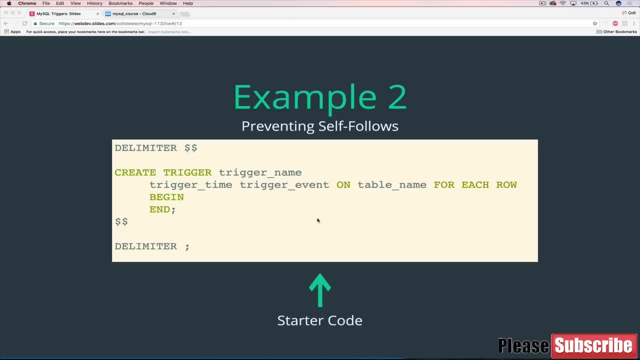 You don't have to do it on the database side of things. You can do it on the client side or in the application side of things. Basically, rather than sending the request to the database to insert a new follow with the, let's say, ID five. 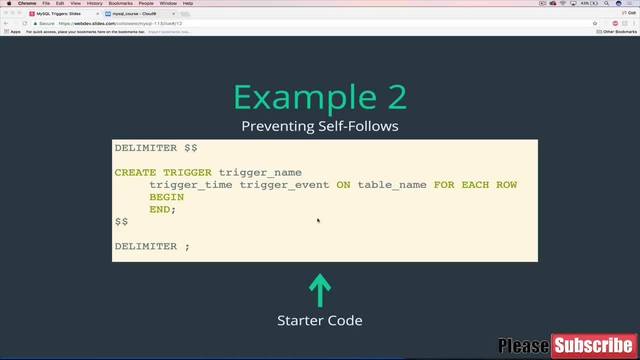 where follower ID is five and follow ID is five. You could just prevent that from being set in the first place by checking on the client side. But there are certain situations where you would want to do this, And one is this case where we're not working with external code. 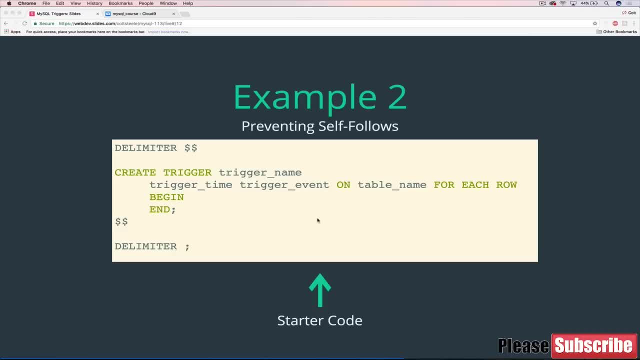 We're not working with another application, We're only doing MySQL. So I'm kind of doing this because a lot of people have been asking about it, But I'm not fully endorsing this as the best solution in actual application, But for us it's really the only one that works. 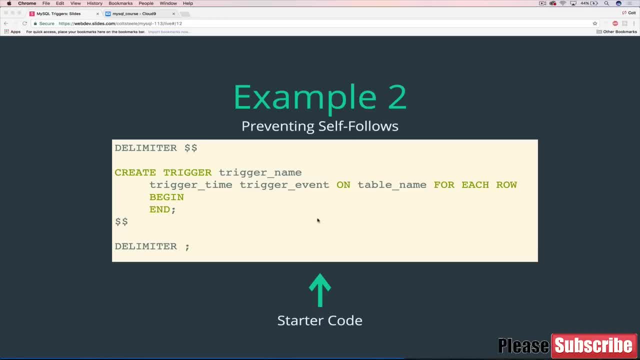 And it's a perfect example of doing a validation with triggers. So what we want to do is just check, basically, when something is being inserted, a new follow is being inserted, check if the follower ID is equal to the follow ID and, if that's the case, throw an error. 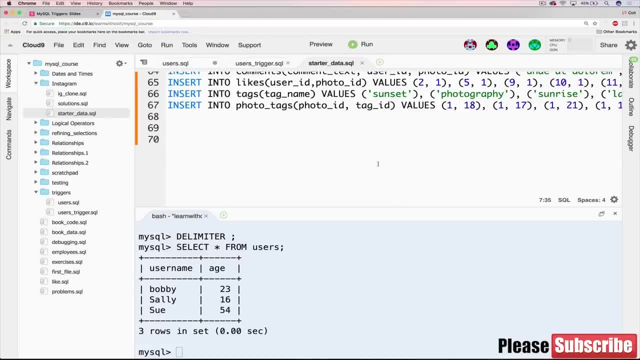 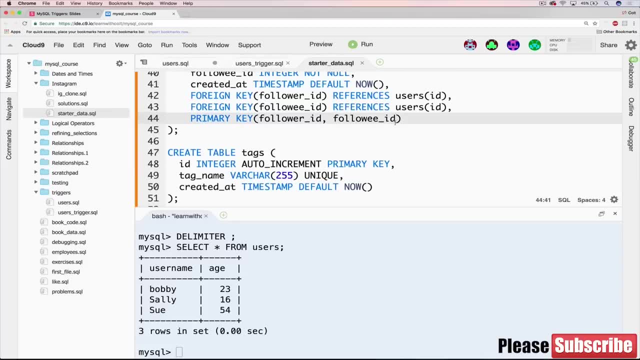 OK, so I'll hop over to cloud nine And the first thing I'm going to do is actually copy over the old starter data file from the Instagram section. Now you can just add this to your existing Instagram database, but I'm going to keep it separate, just so that if people are following along. 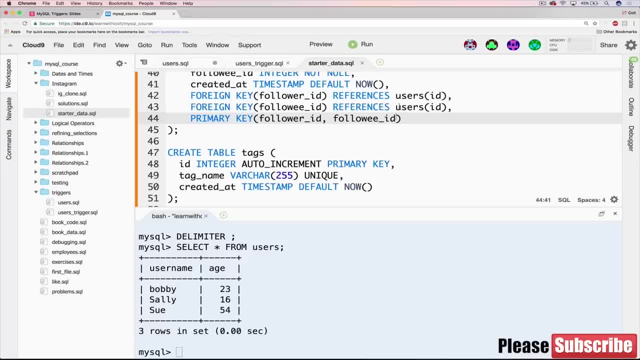 and looking at the code from the previous section, they're not getting confused about this trigger stuff, which they haven't encountered yet, But not all that important. What I'm going to do is just Make a new file here. I'll just call it IG dot SQL. 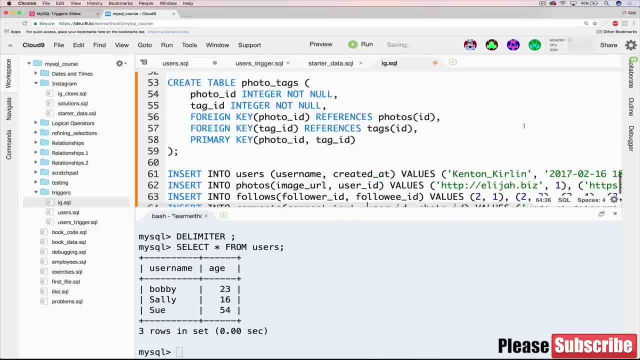 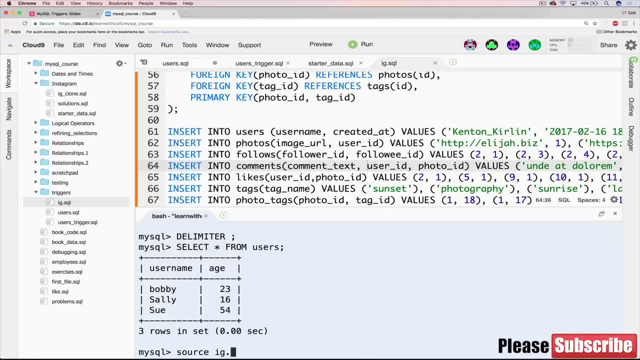 Paste all of the stuff that creates the tables and the starter data. Again, you don't have to do this, You can just work with your old database. But now I'm going to source that file. Source: IG dot. SQL Perfect takes a little bit because we're 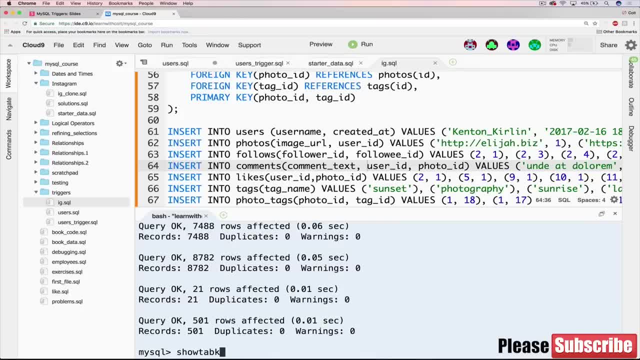 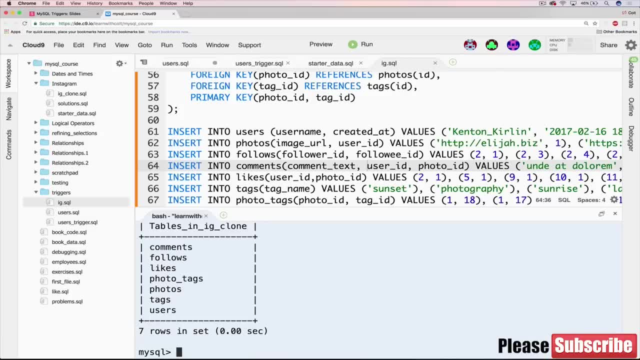 inserting a bunch of rows. but now, if I do show tables- Oh geez, Remember I have a screwed up wrist. I'm blaming that for my typing- You can see we have all these tables. So to illustrate the problem really. 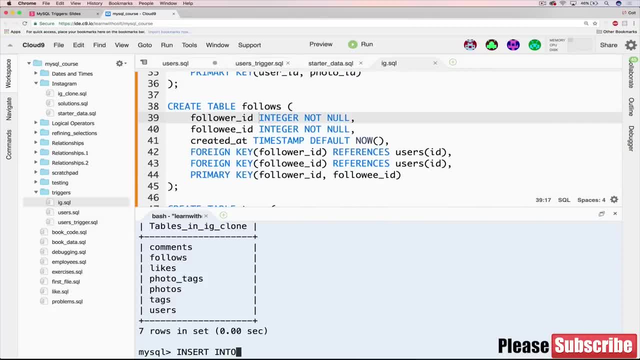 quickly, I could do something like insert into follows And we'll just do follower ID, comma, follow we ID, just like that values And let's just pick an ID. We're just going to assume that someone has the idea, for I don't actually know that for a fact, but I'm pretty sure somebody does. 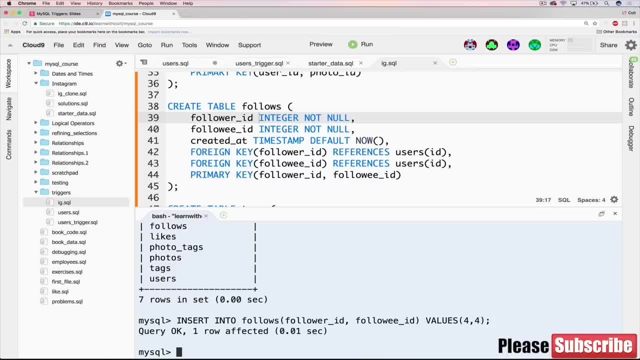 So if we do that, No problem. So our goal here is to prevent that from happening. We don't want someone to be able to follow themself, So I'm going to go ahead and make a new file to write our trigger inside of. 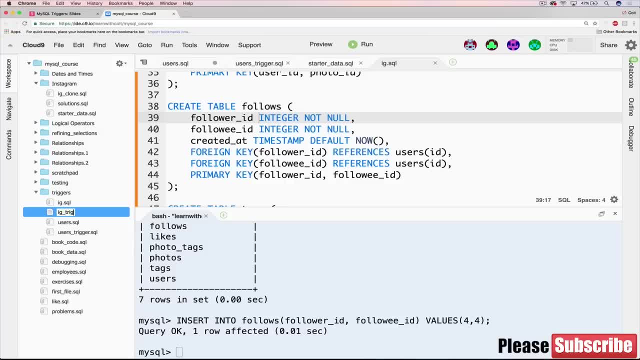 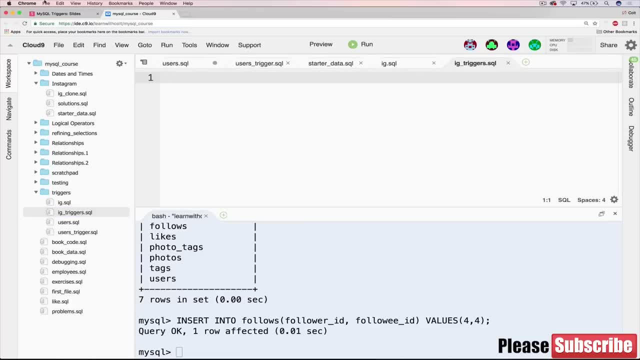 And I'll just call it IG trigger, That SQL or triggers, in case we have multiple later on. OK, and then inside of it I'm going to copy this boiler and get starter code that I provided, just so that we don't have to type all. 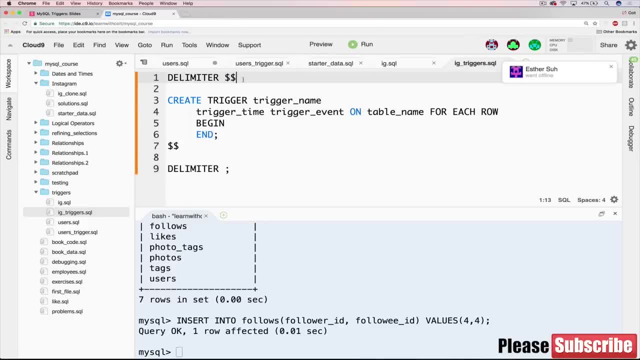 of this from scratch. we can kind of fill in the blanks. So we change the delimiter to double dollar signs, Then we're going to create a trigger and we'll just call it prevent, self, Follow, follows and the table name will start: there is follows. 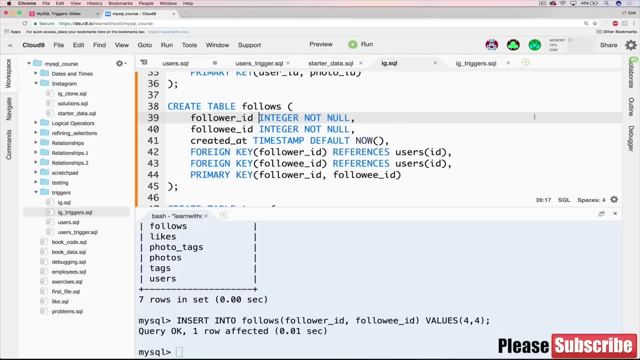 Now the two most important parts are when this happens. basically the time is going to be before or after. and then what event? what change to the follows table? So we know we want to have it happen. on insert: So when something is inserted into the follows table and we want it to happen, 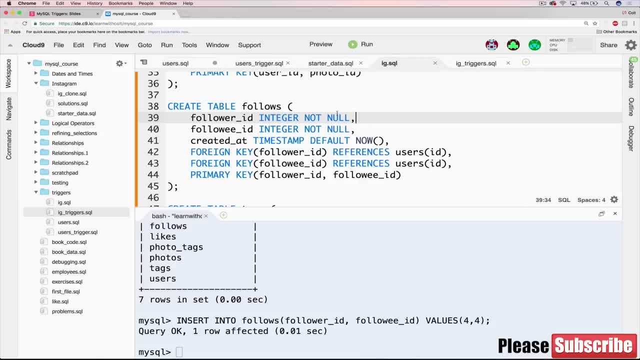 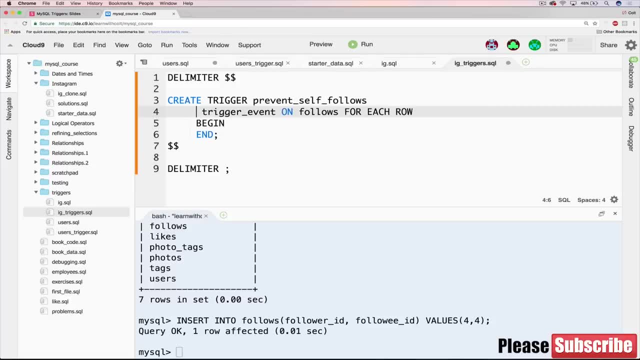 before the insert, because we want to check if we're going to insert it or not. If we do it after the fact it's not very helpful because the data is already in there. So we're going to have before And then the event is insert on follows for each. 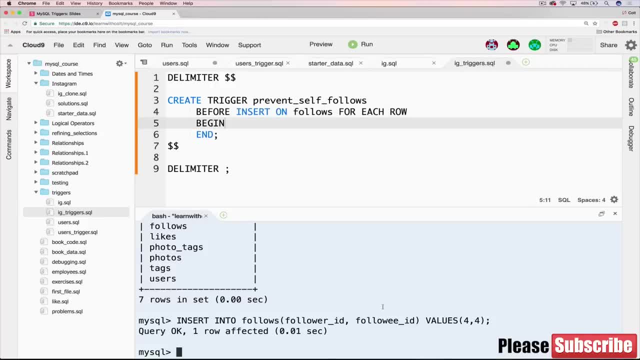 And then, after the throw begin and end, we fill in our code here. So the actual logic here is actually pretty straightforward. All we want to check is if the follower ID of the new- the thing that's attempting to be created- is the same as the following ID: 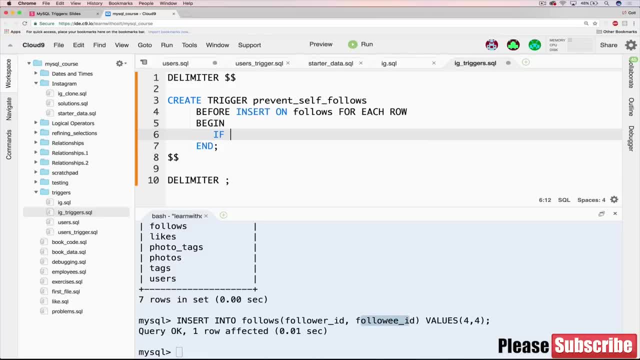 So that's going to be an if statement. We'll have an if and then we can use new dot follower ID. the order doesn't matter. equals new dot follow We ID. if that's true, then we'll have a then. 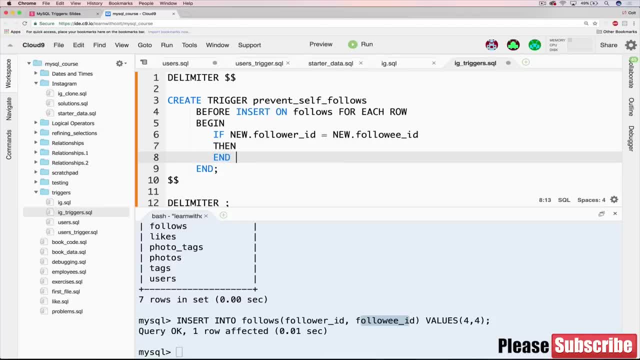 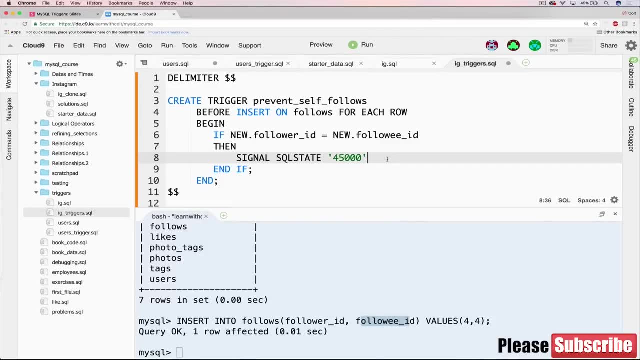 And I'll also add in the And if With our semicolon. so if that's the case, we'll do the signal SQL state forty five hundred forty five thousand and we'll also do set message text equal to, and we'll just say something like you can't. 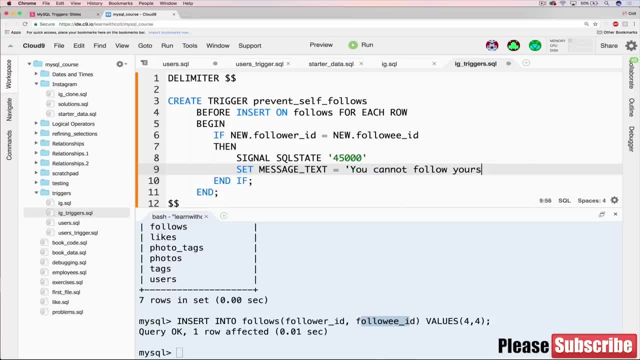 need to watch our quotes there. you cannot follow yourself Just like that And at our semicolon. All right, so we can save that. Now let's see if it works. So to run this, we're going to source IG. 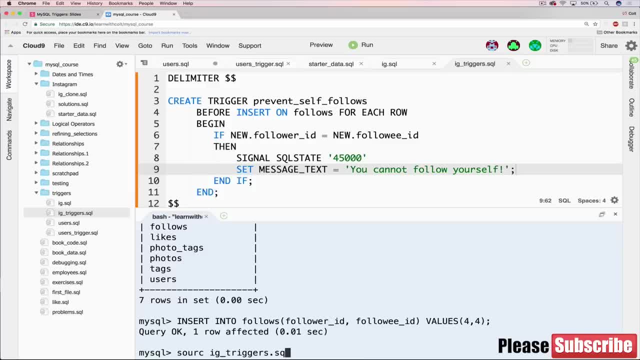 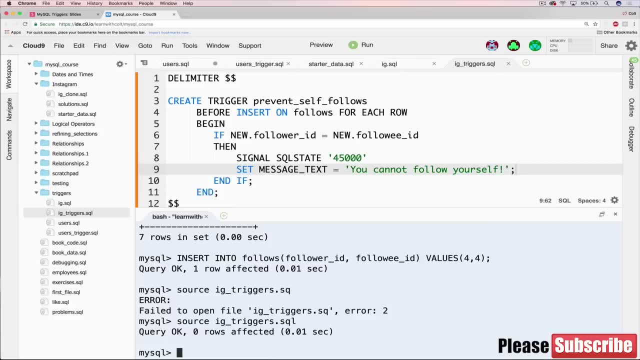 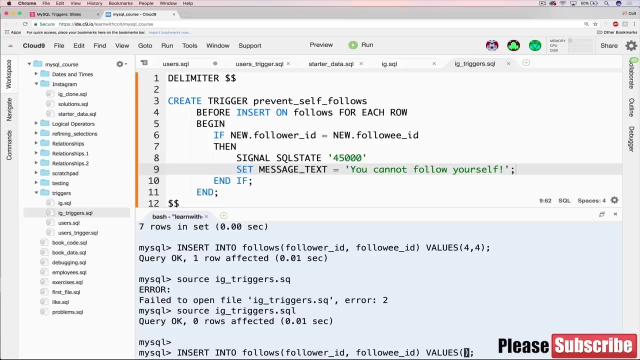 Triggers dot SQL. Make sure we've saved the file first and we spell source correctly, Missing the L on the end. OK, so it looks like it worked. Let's try another insert. instead of four and four, Let's do five and five. 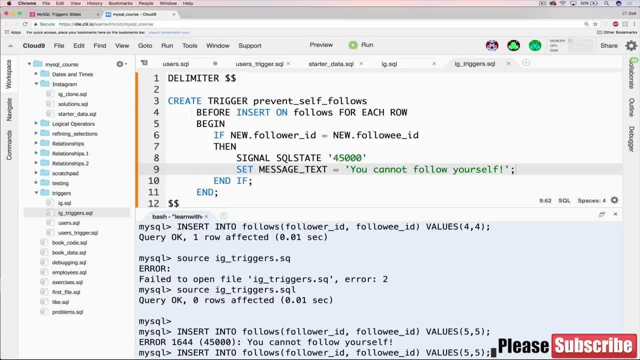 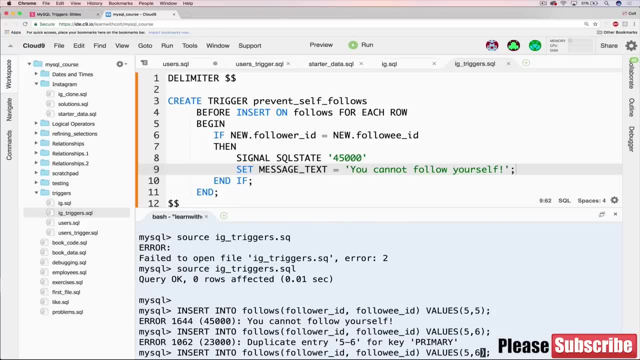 And we get: you cannot follow yourself. Great, That's good. Let's just make sure that we still can follow things how it's supposed to work. Oh well, that's a duplicate entry. How about seven? Oh, come on. 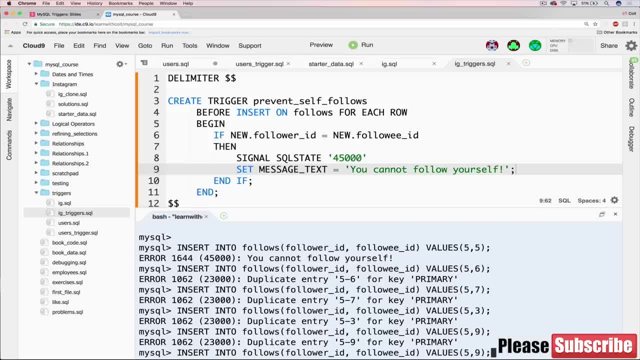 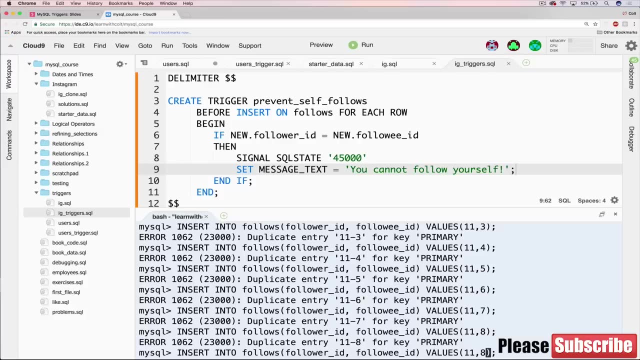 These already follow each other. How about? OK, let me pick something maybe that hasn't followed. a bunch of people. Four comma two: Oh my gosh, They're all following each other. Well, All right, Took me a second, but I went back and looked at the data. 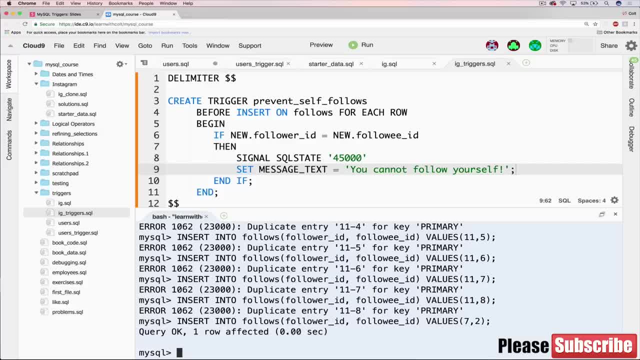 Seems like this should work. Seven doesn't follow many people. There we go, Sorry about that. So basically all of this was a problem, just because we had a lot of people already following each other, so I had to find some combination that wasn't already. 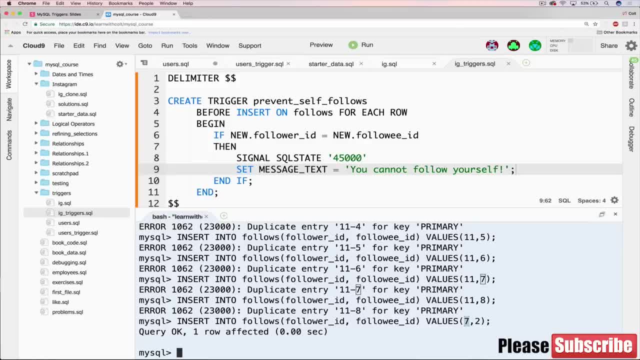 following each other. so seven idea of seven. now is the follower. Two is the following: And that worked. But if we tried to do seven comma seven can't follow yourself. OK, so that's that. The solution is here as well on the slides, if you want to take a look. 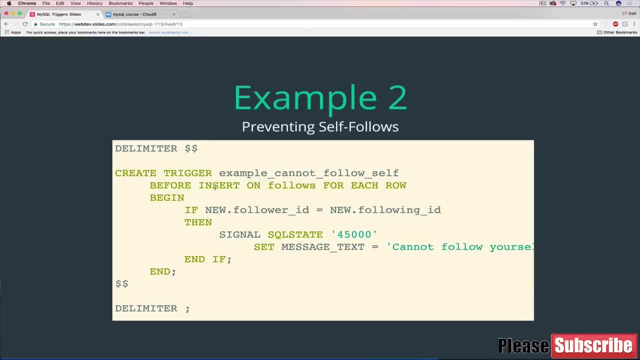 So, to wrap things up, we used before insert again- So that's a common pattern if you're doing a validation- and we used new to compare the incoming new follow entry, the new row, the follower ID to the following ID, And then this is basically the same. 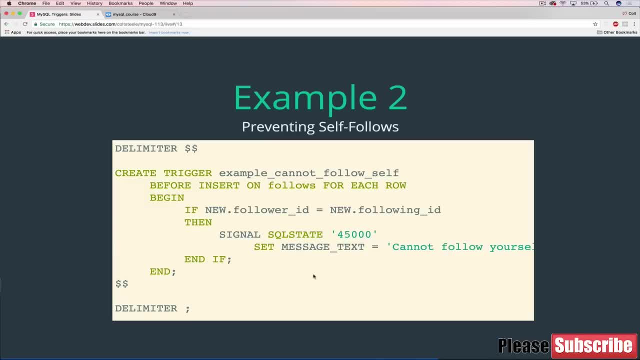 So there's a lot of kind of boilerplate code that you can copy and paste. Hopefully you see that by now. So we have one more example coming up which is a little bit different. It's not so much a validation. We're actually going to be inserting data into another table inside of a trigger. 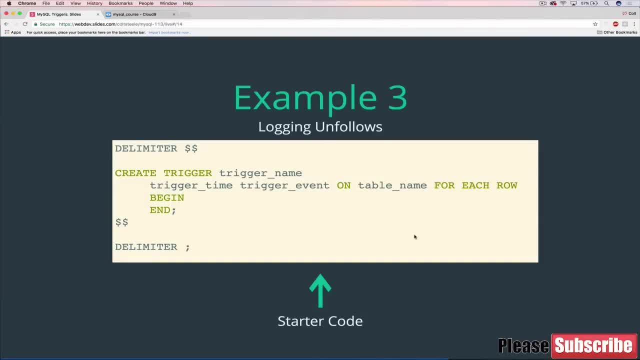 All right. So our final example here, as I mentioned, is a little different. We're not just going to be validating data before it's inserted. We're actually going to create new data based off of another action. So we're working with Instagram still. 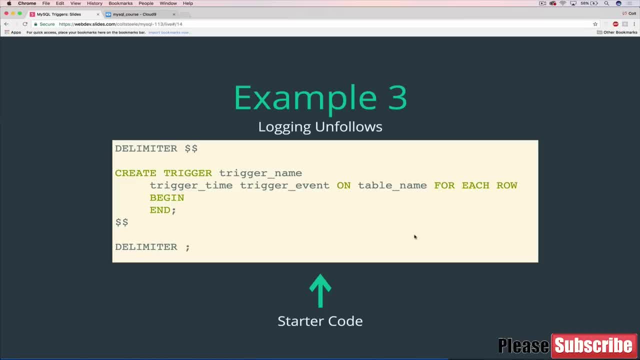 But the idea is we want to keep track of when somebody unfollows somebody else Right now. when a follow is deleted, when that entry is gone, it just disappears and we don't have a record of it, which is typical. That's how most databases work. 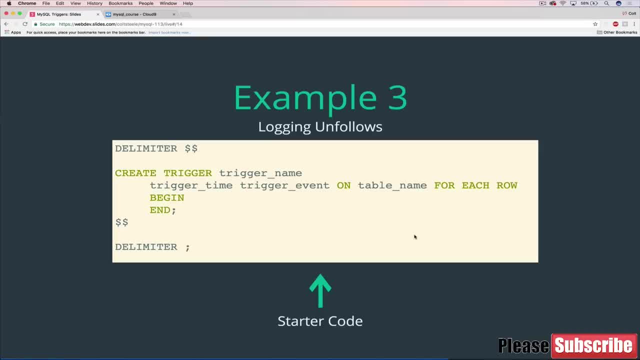 But sometimes there's information that you would want to keep, that you might want to store so you could refer back to it later because it could be meaningful. So in a site like Instagram, if there's a pattern to people unfollowing certain companies or other, 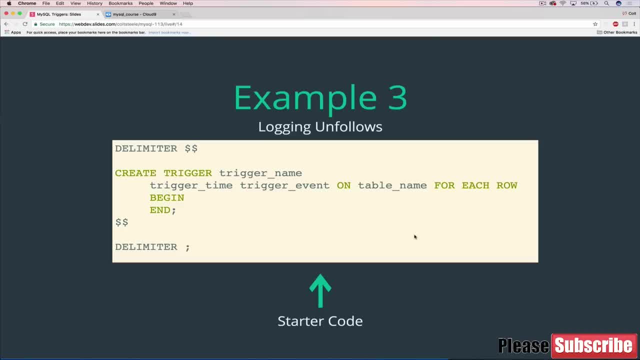 users and you can discern that pattern. that's potentially really important to figure out why people are unfollowing or when these mass unfollow events happen. It's valuable information. So the idea is that, rather than doing something before an insert, like we've been doing here, 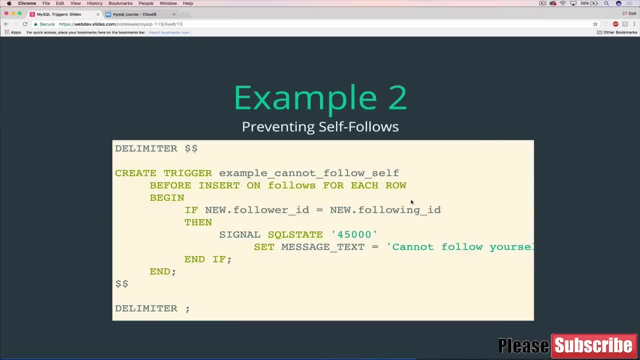 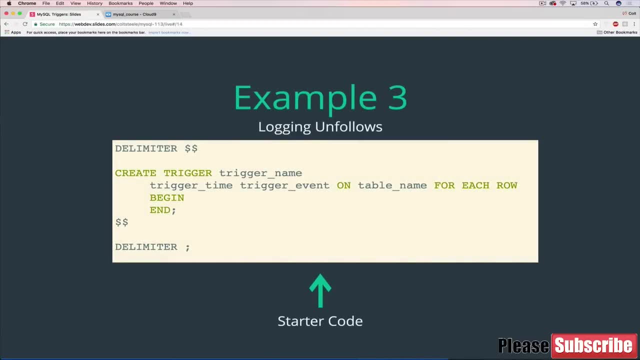 we're going to do something actually after a delete. So after a follows is deleted, we're going to insert a new row into a separate table that doesn't exist yet, So we're kind of going to be transmitting it from one table to another. Now you could argue there are other ways of doing this. 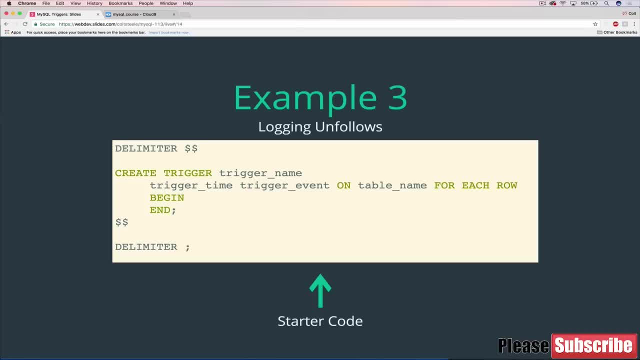 You could. you know, instead of creating a new entry in a table, you could take the original follows table and have a status- active or deactivated, or following and unfollowed or something like that- that you could toggle on and off. There are merits to that. 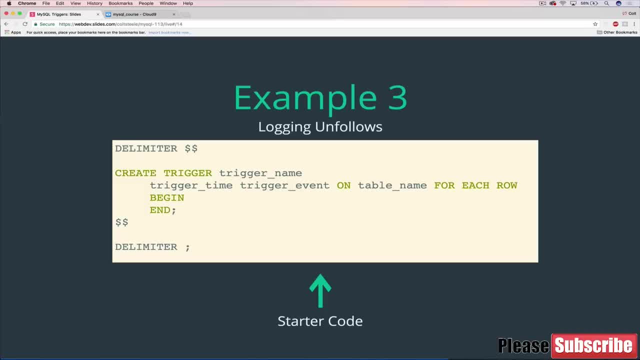 There are merits to both sides, But because this is in the trigger section, it's a great example And it's a really common application. just logging information, logging events that happen is probably the most common use for triggers, So hopping over here. what we need to do first is actually: 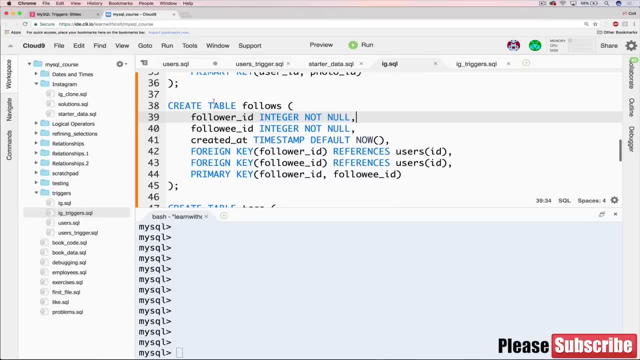 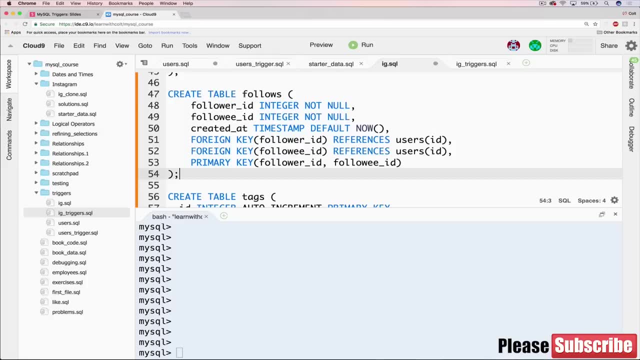 define a unfollows table. so we have our follows table. I'm just going to copy the entire thing And change it to unfollows And we'll keep it as follower ID and follow ID. that's fine created that. everything else can stay the same. 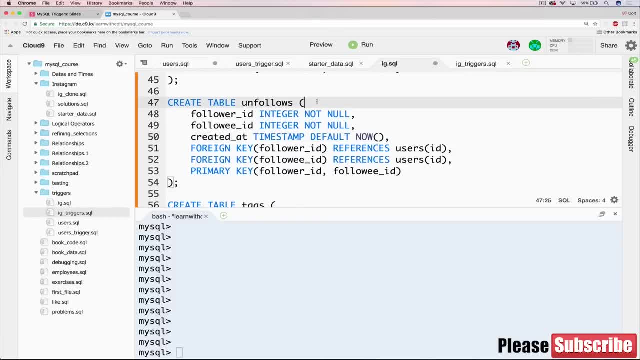 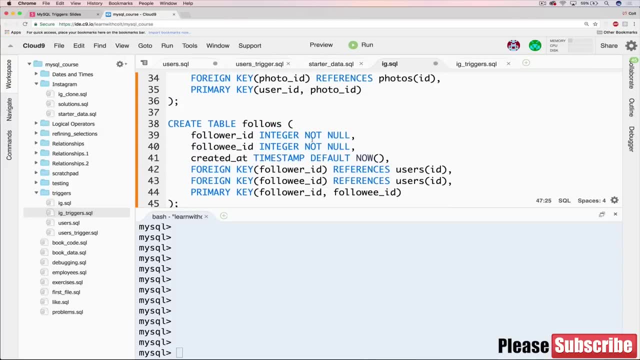 Now we have basically a duplicate table just called unfollows, and it will start off empty. But then let's say, you know someone with ID of five is following someone with ID of six, and then they delete that or we delete it because they've unfollowed them. 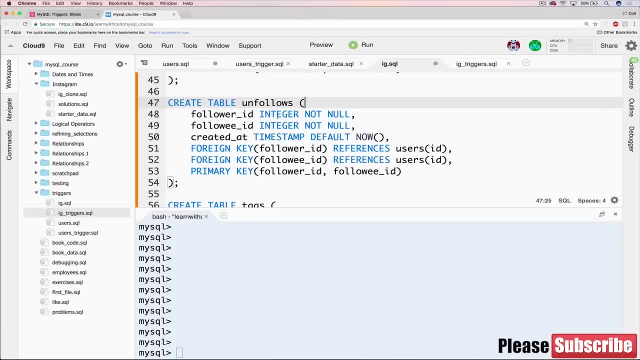 We would then take that and insert it into the unfollows table. The same order: follower ID and following ID are the same, But then we have a time created at for when that event happened, when the unfollowing happened. So that's pretty much it. 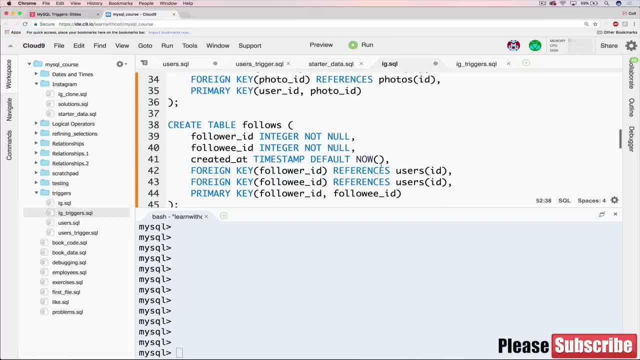 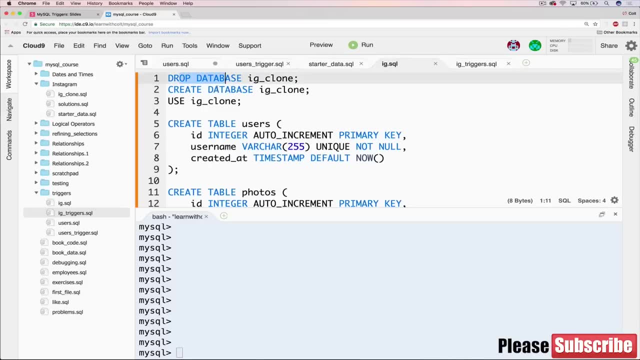 Now what we want to do is have it happen automatically whenever a follows is deleted. So first things first, I'm going to rerun this file. I'm dropping the database, creating it again using the database and then creating all these tables, inserting all this data. 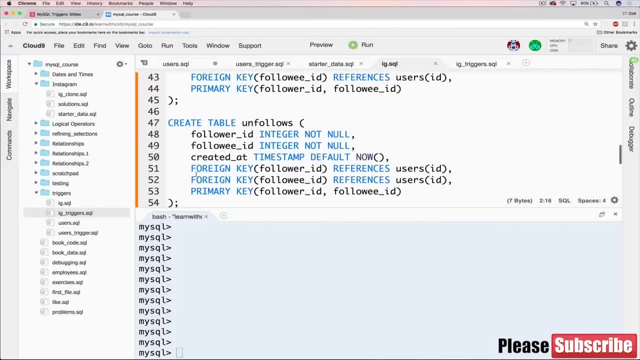 You don't have to do that. If you just want to follow along, just run this code here. Okay, source: IG dot SQL. Perfect, So we've got that new table. If we take a look, Unfollows and it's empty. 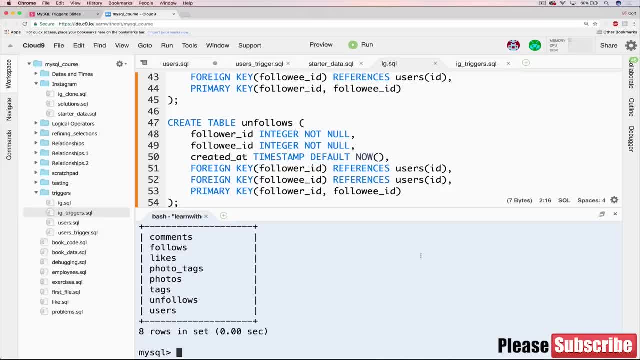 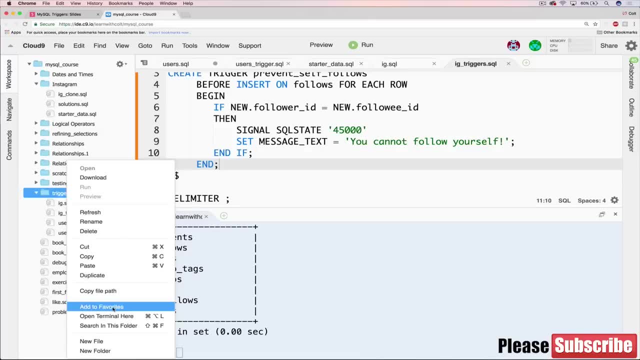 You'll have to trust me on that. So what we want to do now is actually create our new trigger So we could do it in the same file. I'm going to do it in a separate file just so it's easier for you to see if you're going through my code here. 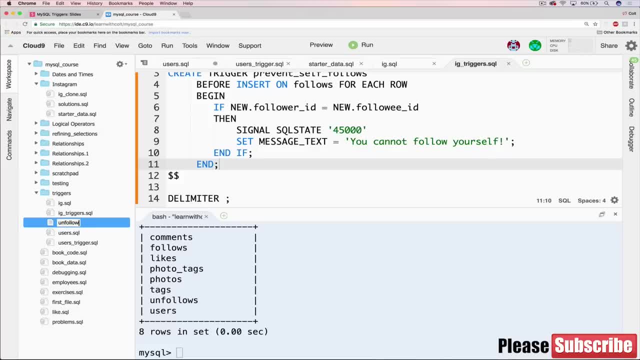 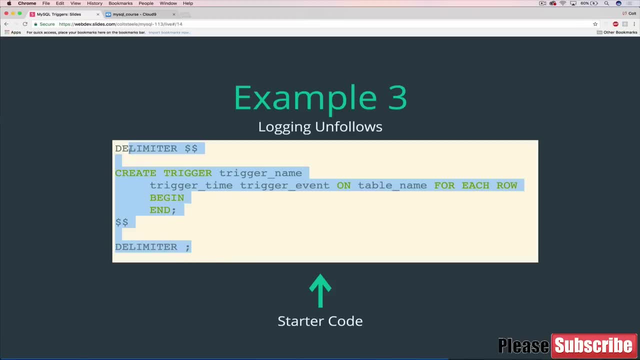 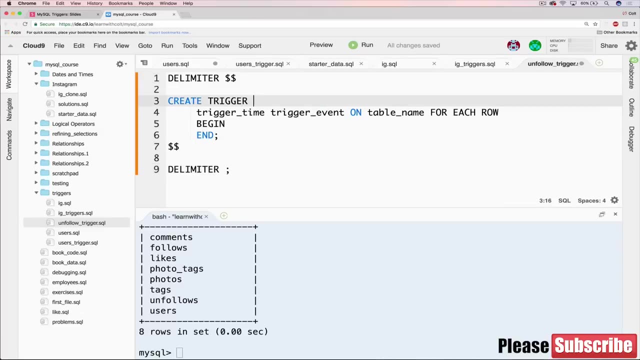 So we'll call this the unfollows trigger, Perfect, And I'll go ahead and copy the starter code again and paste it in. So the trigger name. we could call it anything. Let's go with capture, unfollow or something like that. 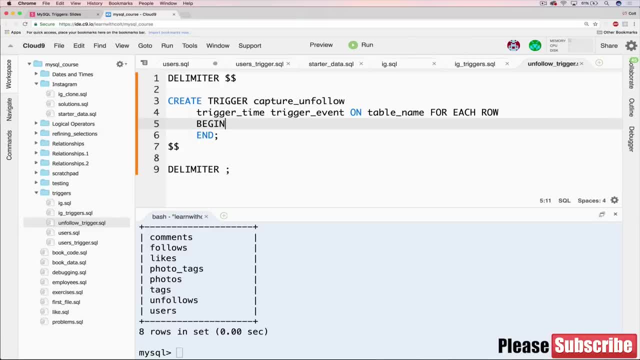 And what we want to do is, rather than doing it before something is deleted, we can do it afterwards because maybe there's a problem, Potentially something wouldn't be deleted. Struggling is a good example, but there could be some situation where the delete doesn't actually go through. 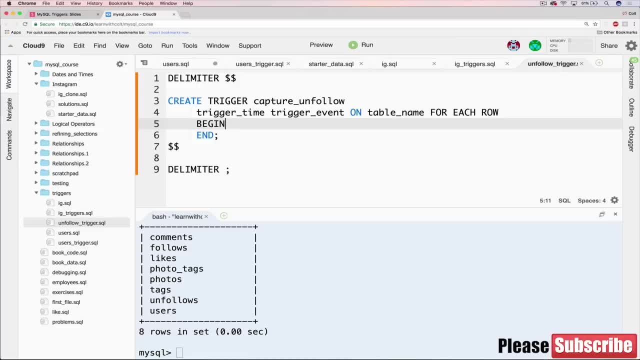 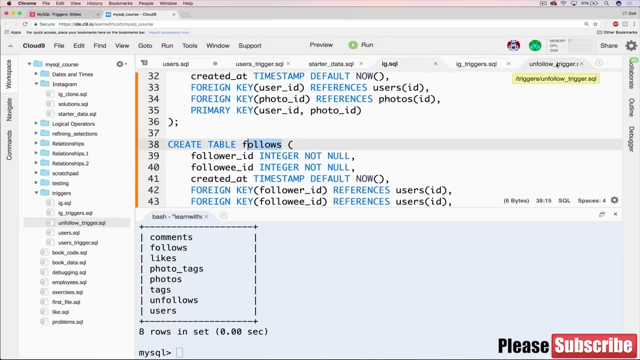 in which case we don't want to create an unfollow, So we're going to do it after something is deleted. So after delete on the table, name is follows. That's our follows table here. So when one of these is deleted immediately afterwards, our code goes in here. 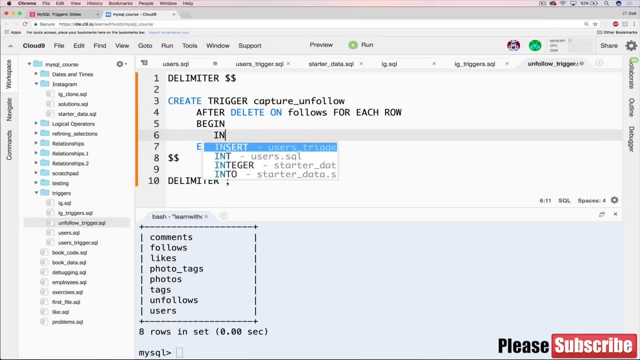 And all that we want to do is insert into the unfollows table, just like this. Insert into unfollows, Then we'll have follower ID and followee ID. There we go, And then our values. And the question is, what are those values? 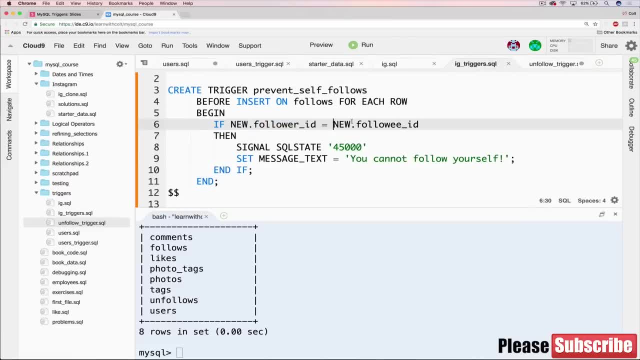 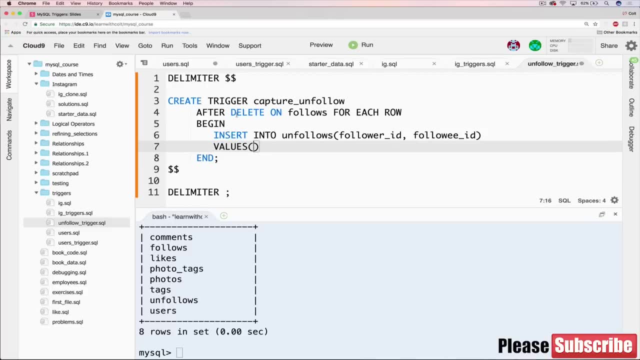 Just like before, where we had newfollowerID and newfolloweeID corresponding to the new row that's going to be inserted When something has been deleted, we have access to old followerID- oldfolloweeID, just like that. 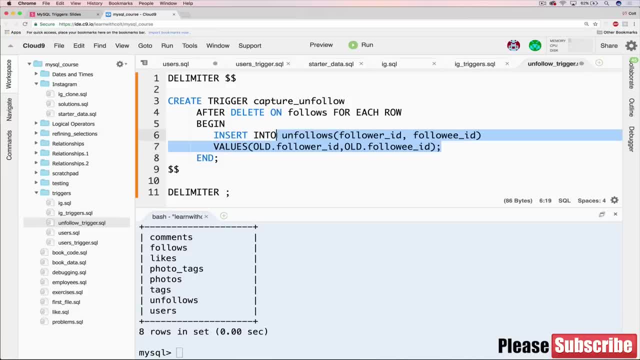 So this works on its own, but I'm actually going to show you another syntax that I like for this situation, which is using set. So the set syntax is another way of inserting something. Actually, we'll just go to my solution to show you. 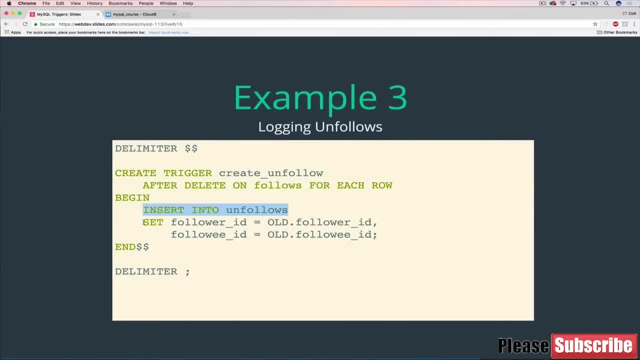 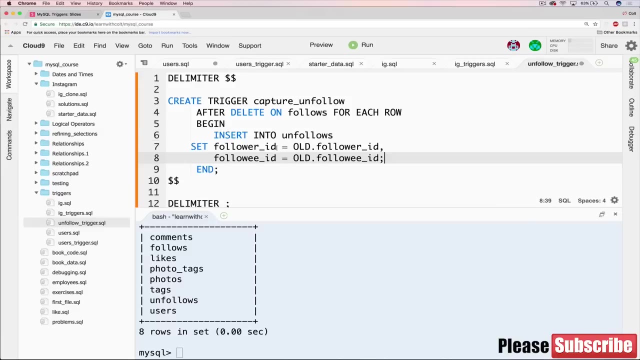 It looks like this: Insert into unfollows And then we have set: follower ID equals oldfolloweeID, comma followeeID equals oldfolloweeID. So it's really up to you what you prefer, but I just wanted to show this syntax. 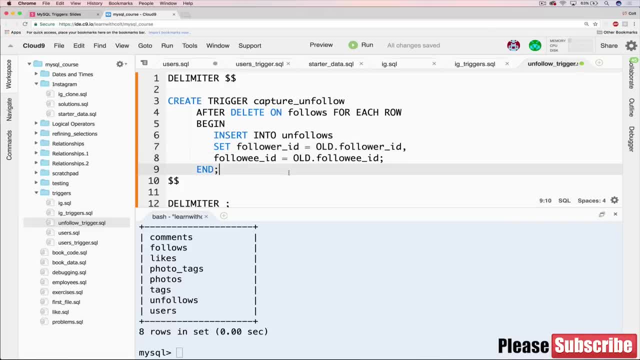 There we go, Just like that. So essentially, all you're doing is using an equal sign to assign them rather than values, parentheses- that old syntax that we're used to, So I'm just going to mix it up here. But, to be clear, you absolutely can use the other. 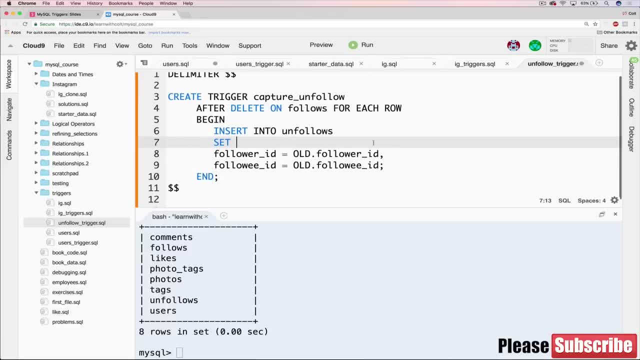 example as well the typical insert. So we don't need an error message or anything here, because this isn't a validation. We're not responding with something. We're not preventing something from happening. All that we're doing is connecting these two tables so that, when something is deleted from follows. 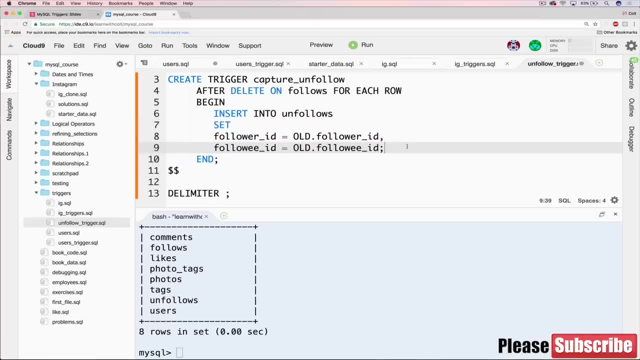 something analog is created in unfollows, which, as I said, is a pretty common situation, not follows and unfollows, necessarily, but capturing kind of metadata or capturing other information based off of SQL. happenings, if you will. So events, things changing being deleted, updating that you're then capturing and 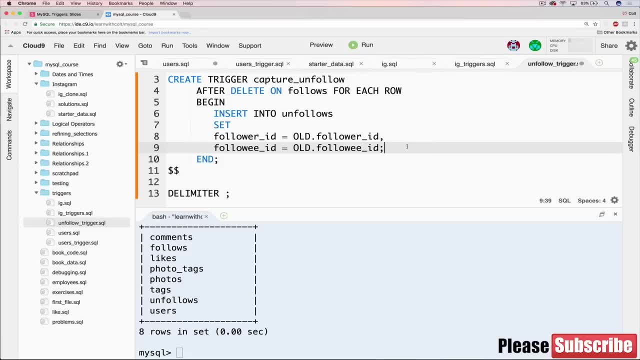 logging somewhere else so that you can refer back to it. So you usually don't just do this willy nilly. Typically there's a reason you want to store that information, Otherwise it can- kind of it can- get bloated very quickly. 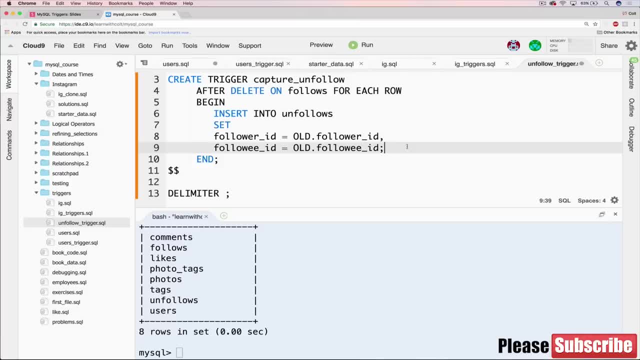 especially if you have a lot of triggers going on. I'm actually going to spend a couple of seconds at the end of this section with some advice about when and how to do that. I'm actually going to spend a couple of seconds at the end of this section with some advice about when and how to do that. 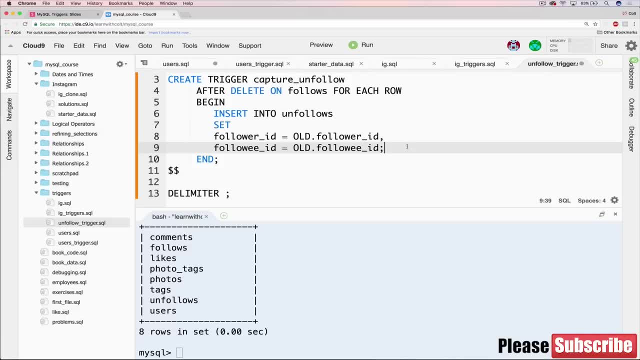 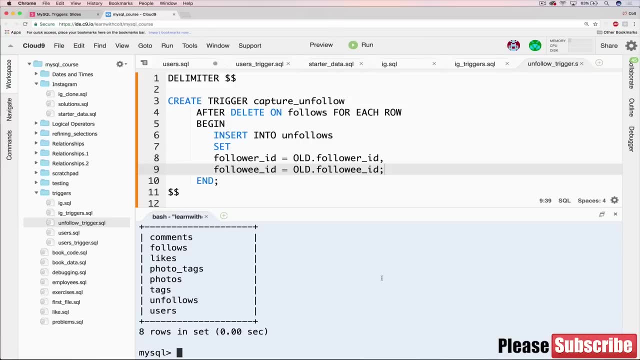 When to use triggers and when not to use them, and how they can get out of hand. But for now this is perfect, So let's save it. Make sure we don't have any syntax issues And let's see what happens. So we'll do. source. 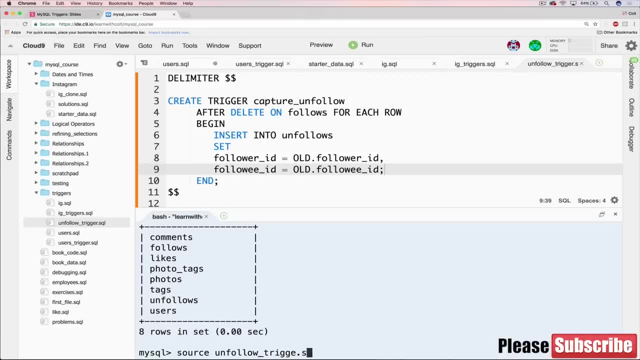 Unfollow trigger dot SQL is the name of the file. Looks like it worked, so let's verify right now. select star from unfollows. Looks like it worked, so let's verify right now. select star from unfollows. Nothing there. 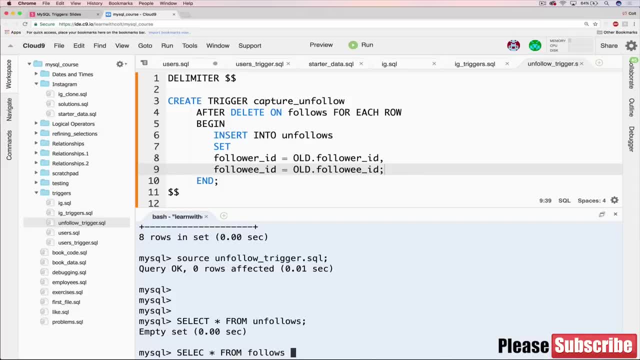 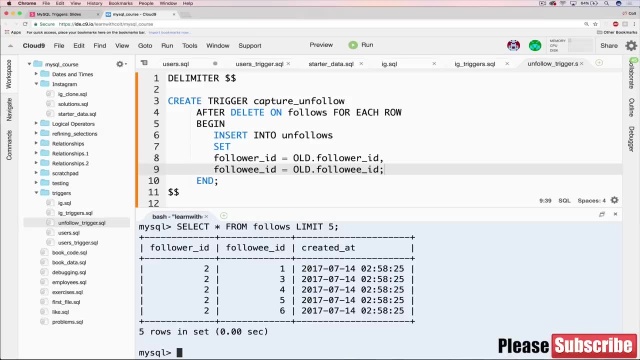 Let's do a select star from follows And let's limit it to five, If I can spell that correctly: select OK. so what we're going to do is say that follower ID two unfollows person with ID of one. So we're going to delete this right here. 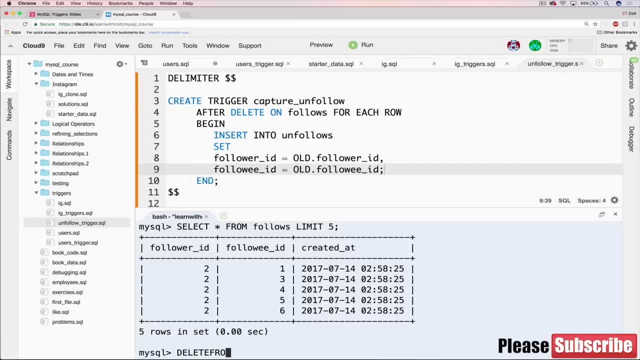 So let's do it now. We'll do a delete From follows where follower ID equals two, and we could just leave it at that. And now we delete all of these that have follower ID of two. So we'll do and follow E ID equals one. 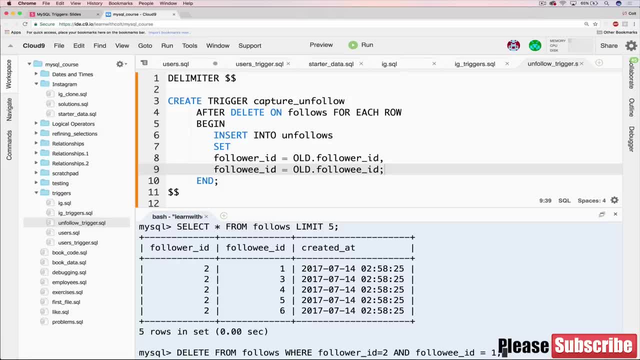 Need that D there, There we go. OK, so it should be gone. if we select it Now, it's gone from there. And if we looked at unfollows, there we go. We now have follower ID two. follow E ID one. 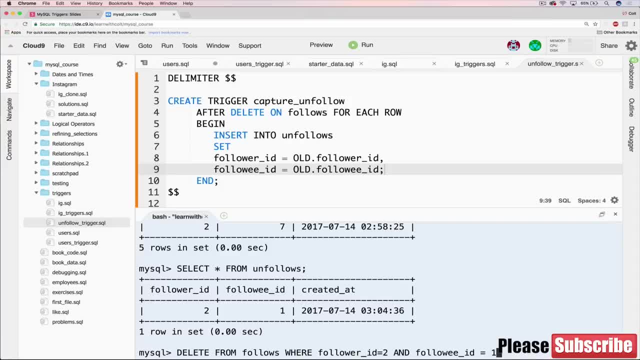 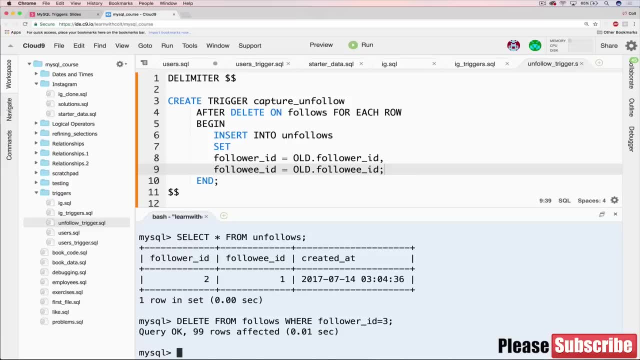 So just to show you that one more time, let's go ahead and delete all follows where follower ID is three. So that should be quite a few 99.. And now, if I look at all unfollows, we have 99 new entries. 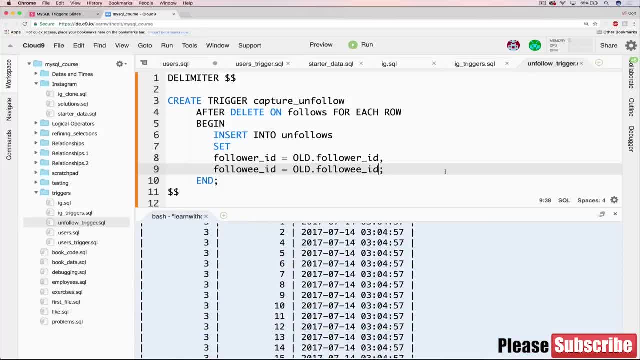 So pretty cool, Very easy way to kind of transfer that data over into another form. And you're not always strictly duplicating data like this. Sometimes you're summing data together, So when something is inserted or deleted, maybe you're keeping a tally in another table somewhere. 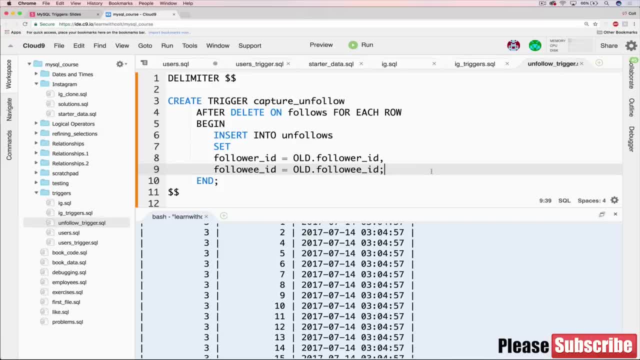 Maybe you're keeping a total. If you have a shopping cart, you have a cart table and then you have your items or your products table And any time a product is entered into a cart, any time a new product is created, you're going to update the total, and you could do that using a trigger. 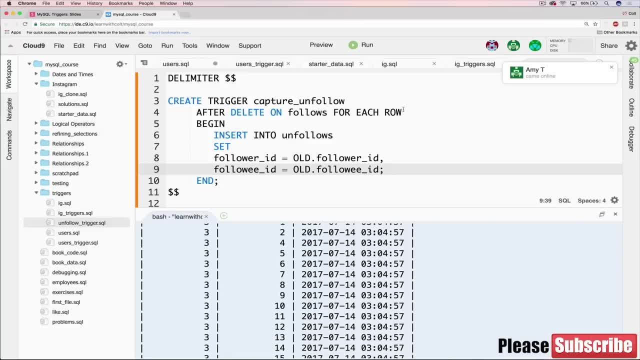 As well. So it's not just copying exact data, like we're doing here, from followers or follows and transmitting it identically into unfollows. But that's a simple example that makes sense in the context of our Instagram data. So that wraps up kind of what I want to do with triggers. 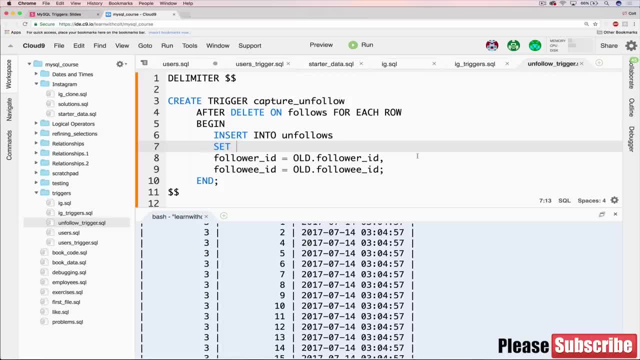 Hopefully you see some of the possibilities around them. The next video is going to be pretty quick, just talking about how you can delete triggers, how you can view your triggers, kind of managing them, And then we'll also talk a little bit about 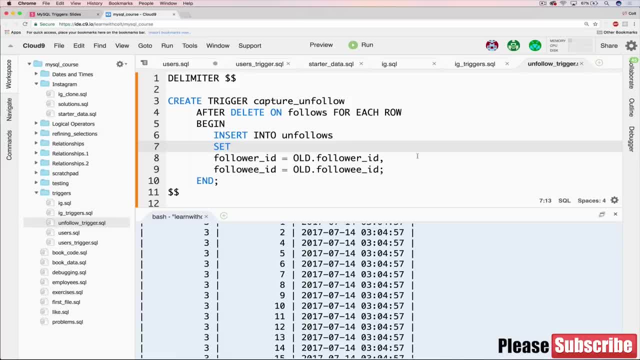 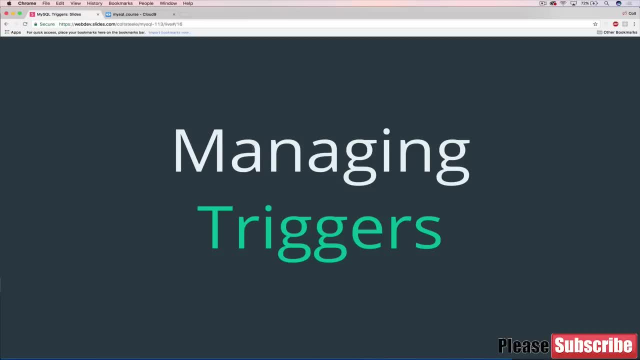 kind of a warning around triggers. So I'll see you then. All right, So we've got one more video here, And this has to do with managing triggers, which sounds a bit like a chapter in a self-help book, But really it has to do with how we make. 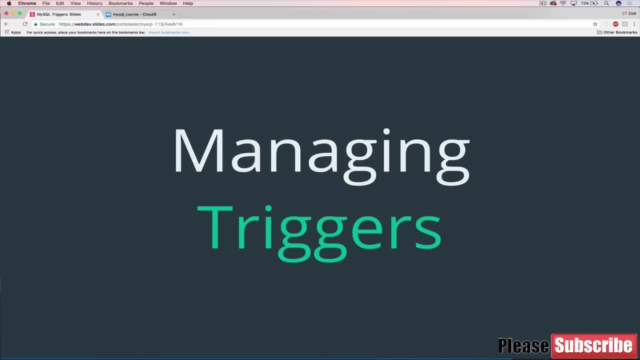 sure our triggers are working and mainly delete them. So this is where the name of our trigger comes into play, And then also I'll end with a quick warning about triggers. So the first thing that we can do is just list the triggers that exist in a database. 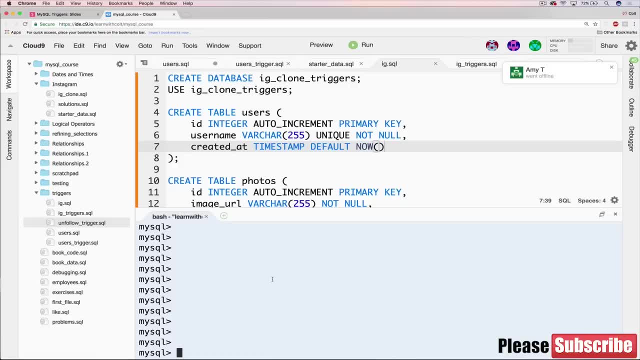 So we can just use Show triggers to see what we have going on. And I'll warn you- this is not my warning I already talked about- but I'll warn you that what you get when you run this is kind of a mess to look at. 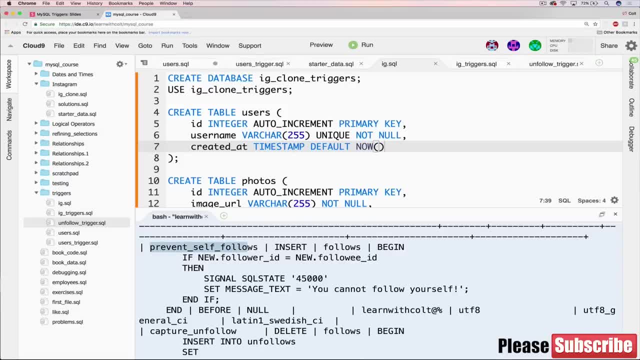 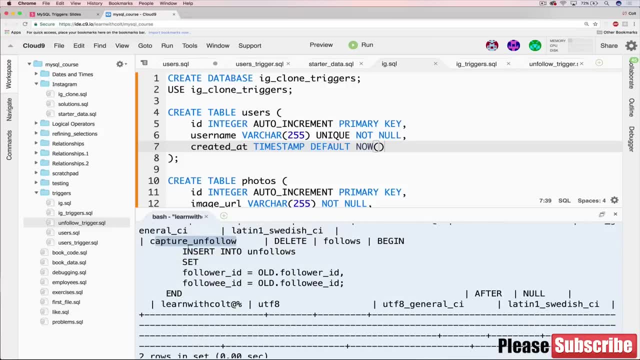 But we can see, we have in our Instagram data. we have two triggers: prevent, self follows- and then you can actually see the code inside of that trigger. And then we have capture unfollow, and you can see that code as well. And if I switched over to the other database, 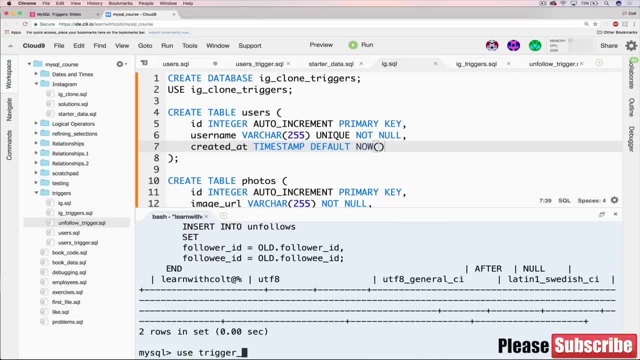 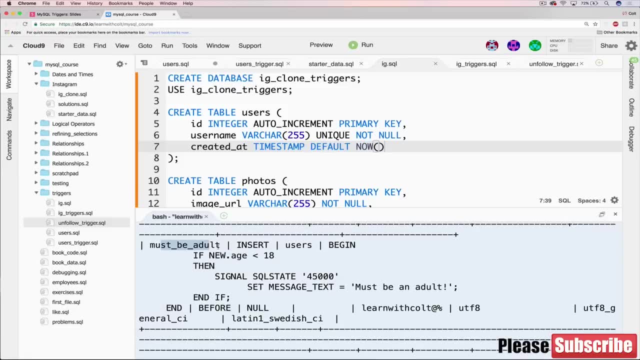 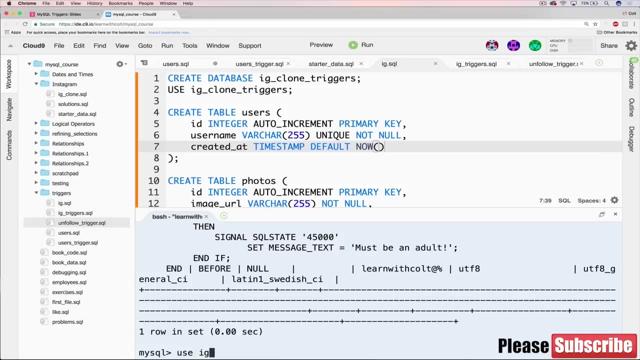 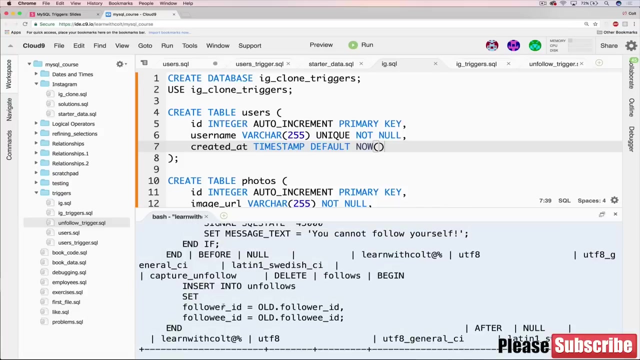 I believe it was use trigger demo And I do show triggers. We have one here. This is our must be adult, All right, So we have that. I'll switch back to my Instagram: clone OK, and do our show triggers, just to make sure they're still there. 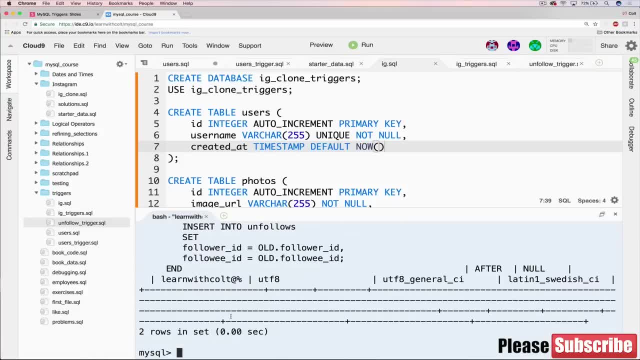 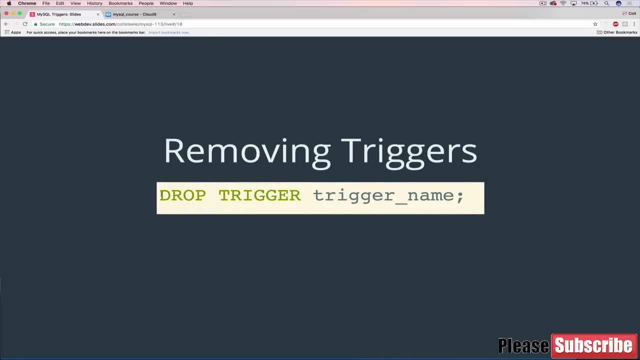 They shouldn't go anywhere anyways, but we've got two of them, OK. so that's pretty much it to listing them moving on. So if I want to remove a trigger, it's pretty simple. It's drop trigger and then the trigger name. 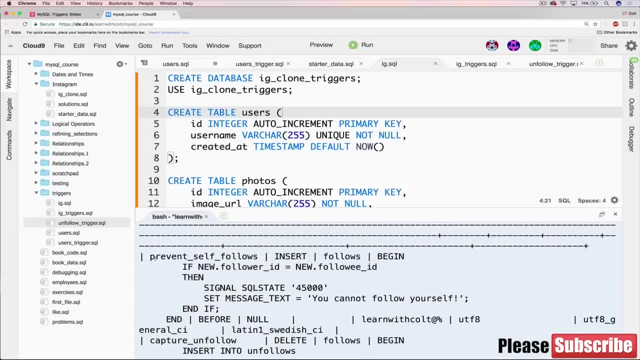 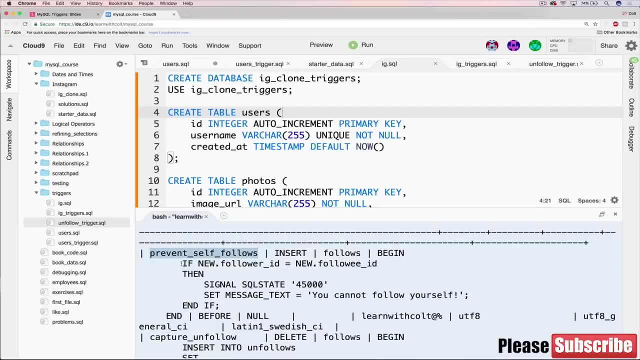 So let's go back. Let's say: I want to remove this, prevent self follows. I want to allow users to follow themselves, So I want to get rid of that. I'll just copy the name, just so I don't have to type it. 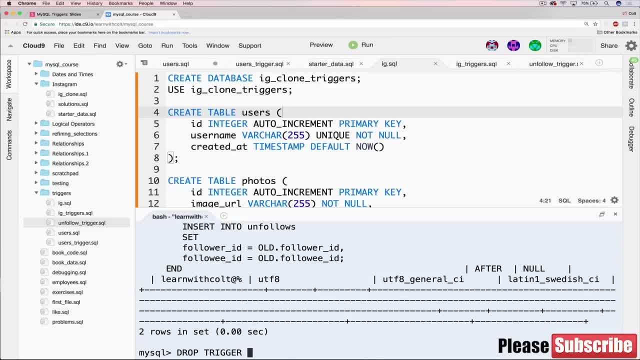 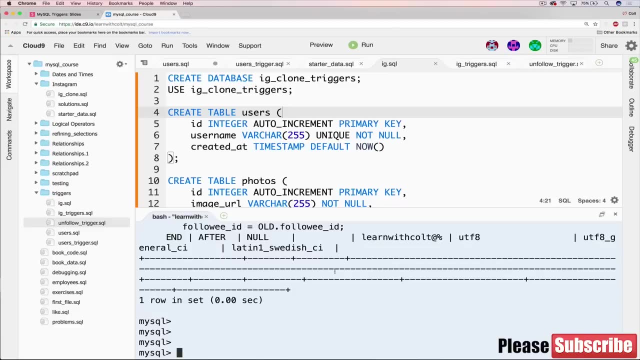 And we just do drop trigger, Prevent self follows And if we do our show triggers again it's gone. And just to verify that it works, it's not just deleting the trigger from show triggers. Let's try and trigger it, if you will. 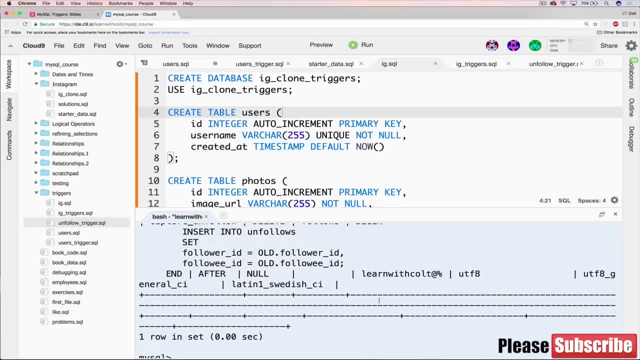 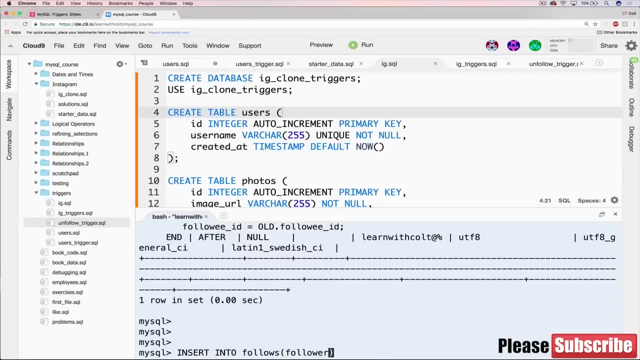 with something that would have caused a problem or thrown an error in the past. So insert into follows. And we have follower ID, follow We just the worst part. So let's insert something where they're the same. How about seven and seven? 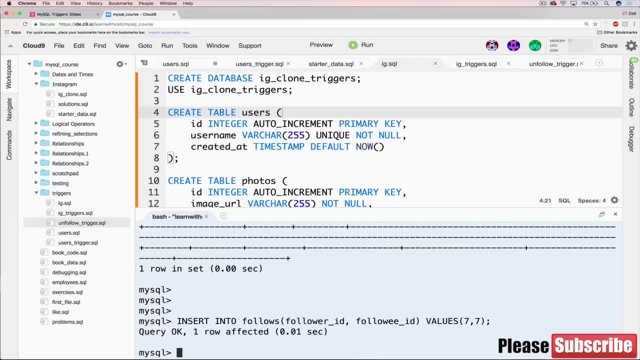 No problem. So in the past that would have been a problem because of that trigger, But it's now gone OK. so that's really all there is to managing triggers, or at least all that I'm going to talk about here. we can look at them using show and we can delete them using drop trigger. 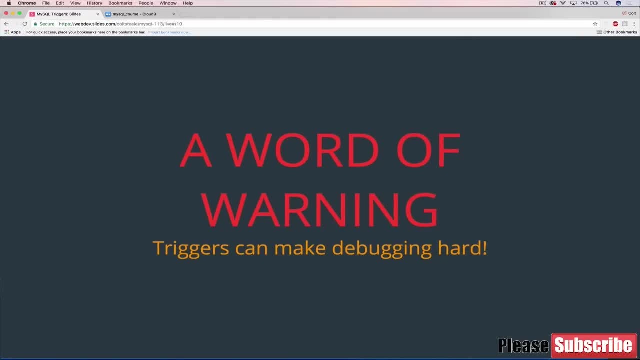 So that brings me to the last thing that I warned you about, which is I wanted to just briefly briefly address a potential hiccup with triggers. This is kind of a concern that a lot of developers have, And it has to do with debugging code. 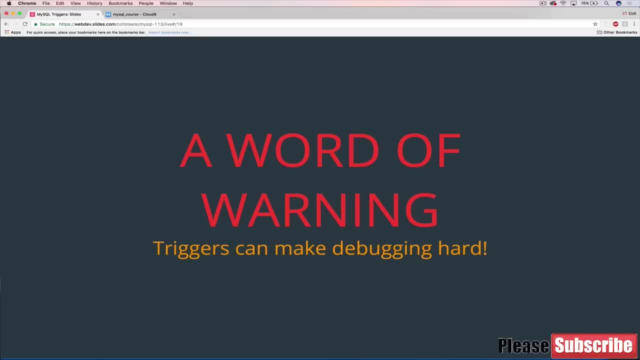 debugging applications that make use of triggers in your database. So imagine that you're a developer on a team with a bunch of people and something's not working how you expect it to. Let's say, when you insert something into a table, you realize that actually two items are being created for some reason, and you have 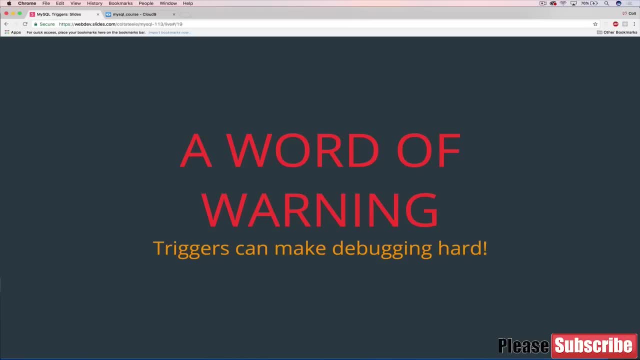 no idea why And you might think: OK, maybe that's something happening on my side of the application, maybe that's my code, that something is wrong with our logic on the front end, with our, let's say, objective C code. 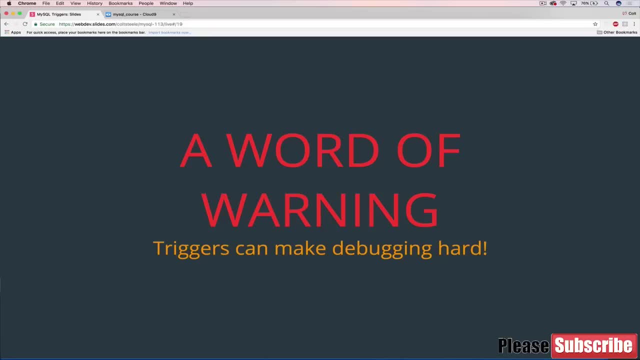 And you could scour that forever, but you would actually never get to the core of the problem if it was because of a trigger. And triggers are kind of stealth little bugs waiting to happen because you have no way of identifying that something is happening because of a trigger. 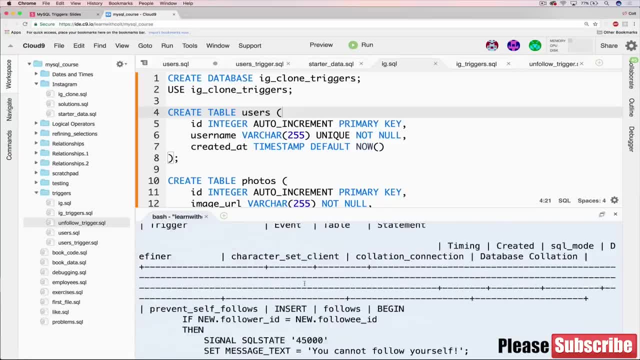 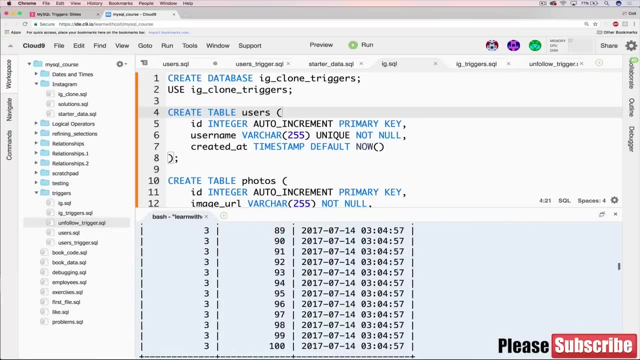 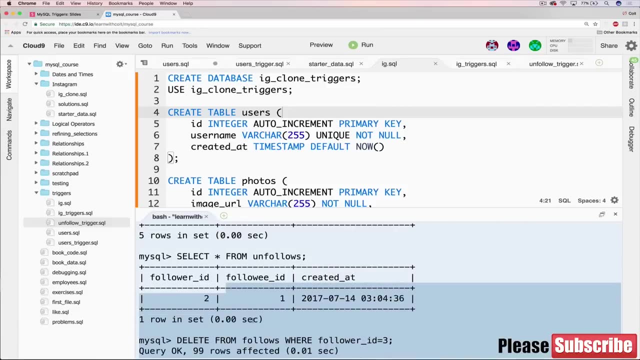 It's behind the scenes Like: remember, go back here with our unfollow If I can go find that way back here. Oh boy, where is that? Here we go Here. we had ninety nine entries created automatically, when all I did was run a single line of SQL to actually delete things. 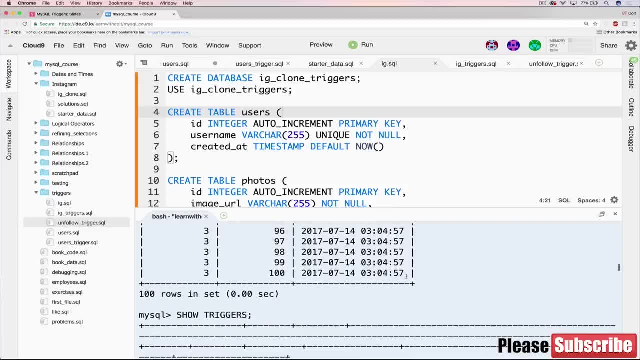 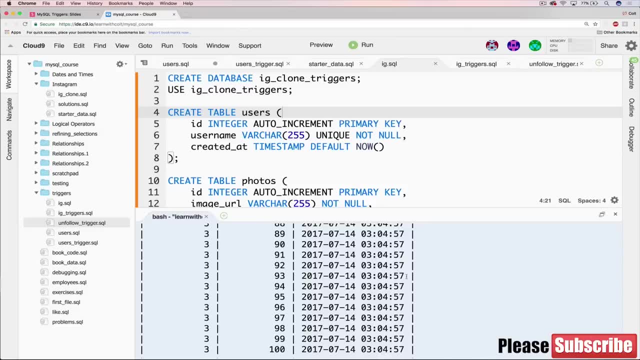 It ended up creating ninety nine things Now. we knew that was going to happen, but if you have a bunch of triggers and somebody doesn't know about them on the team or you forget about them, it can make things difficult to debug because it's basically magic happening. 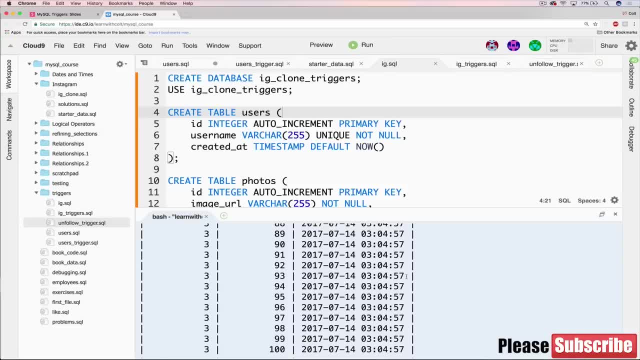 behind the scenes, things that are hidden. Typically, when you're debugging, your code is up in front of you. You can see where the problems are happening. So triggers cause problems sometimes because of that, And the other thing I would say is that 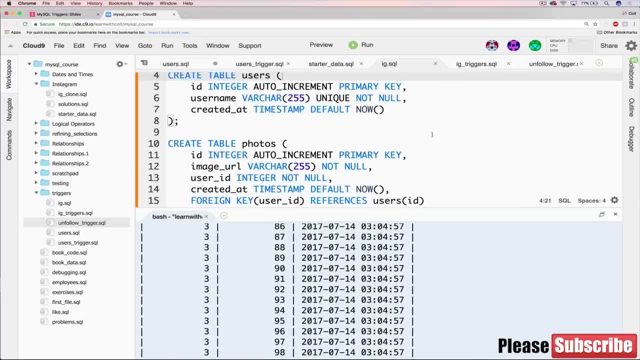 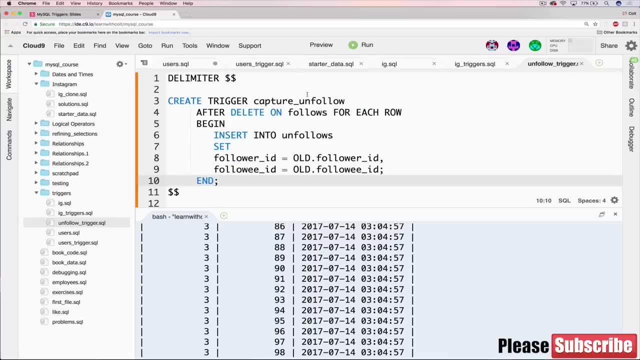 some people have a tendency to chain triggers together. So with our unfollows example you could have another event trigger. So let's say Here when a follow is deleted, we're inserting into unfollows. We could have another trigger for when 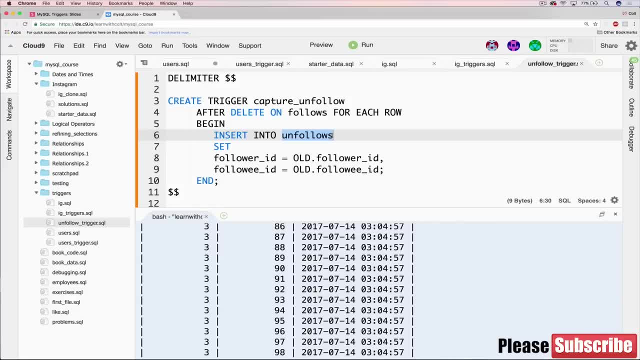 something is inserted into unfollows to do something else and you can chain them together and there's actually situations where, believe it or not, that actually makes sense, but it's kind of frowned upon by a lot of people. So just be conscientious if you're using a lot of triggers.